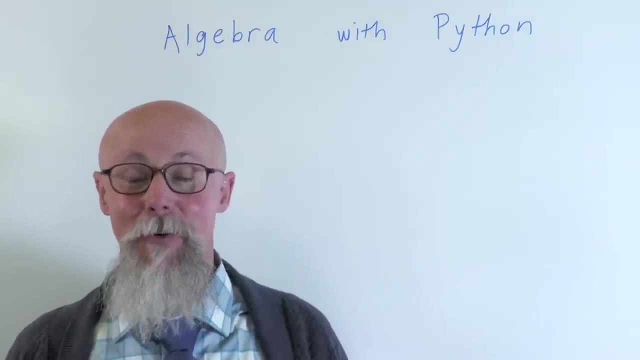 the Google Codelab app, and then you have access to each of these notebooks on your phone. So, you know, you can make your own, like, you know, super calculator that you have access to on your phone, you know, solve all kinds of things, you know, and that's great, You know. 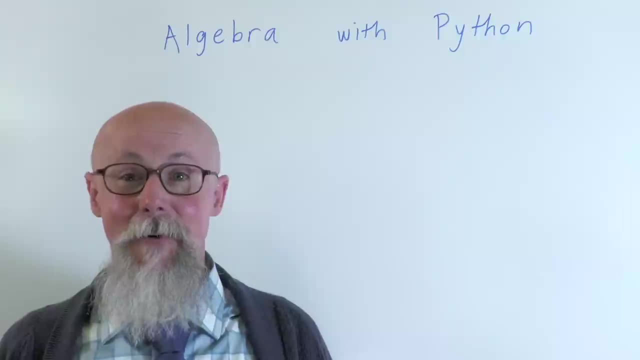 building these resources, but also understanding how to use them so that, as you go further in math and in writing code and eventually leading up to you know, working in data science, that you really understand these concepts and you know how to use all the formulas that you're. 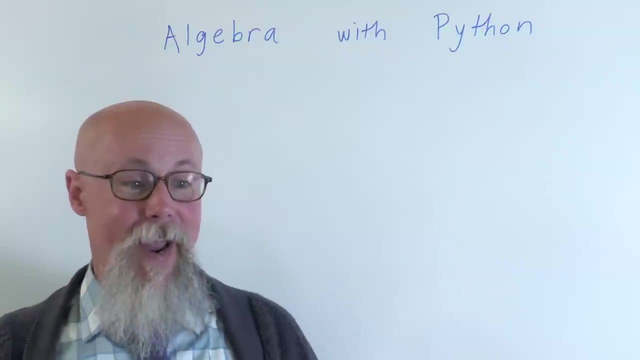 creating. So that's really that's the idea, That's what we want to do, And each unit is going to be a lot like this. I'm going to talk about the math. you know, we'll do some things on the board and then we'll flip it and we'll look at how to do that with code. 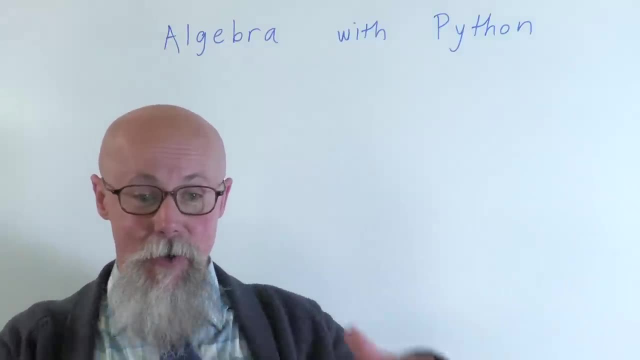 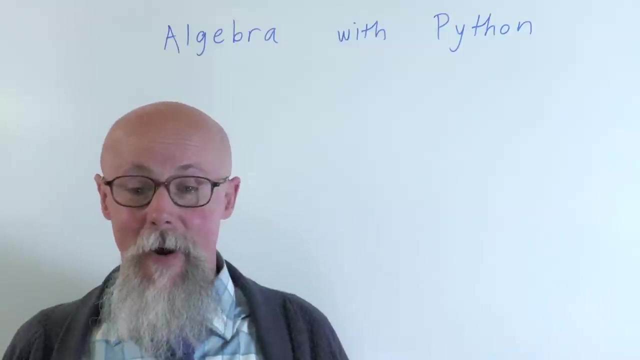 I'll include all the resources for you And then, in addition to the core concepts, in each unit. the next thing, then, what we'll do is I'll have another video or two extra working, working through the problems, So you know, you know how to write the code, you're building your resources, And then we'll just work through a bunch of extra. 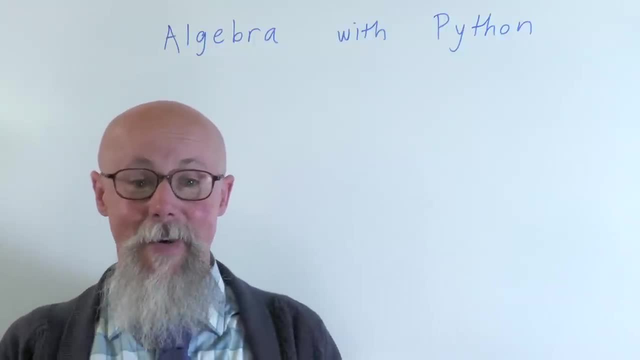 problems. you know putting this into practice And it'll be really great. You know, you'll learn algebra, you'll learn code And you'll have all these skills under your belt that you can use for a lot of other things, And we're going to build upon these in future courses, So I hope you enjoy. 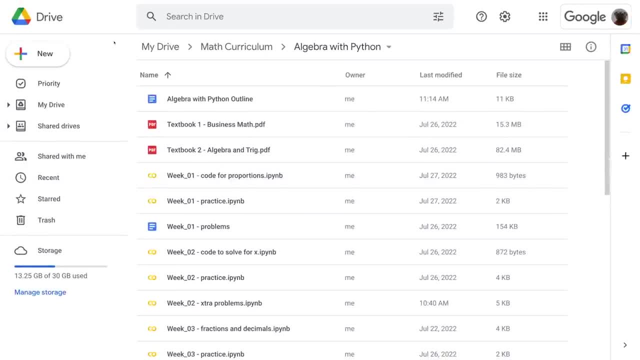 Okay, so let's look at how to set up Google Colab in your Google Drive. So in your Google Drive- hopefully you have it organized in folders And you know you have a- you'll set up a folder for this course. That way, you know, you can have all the. 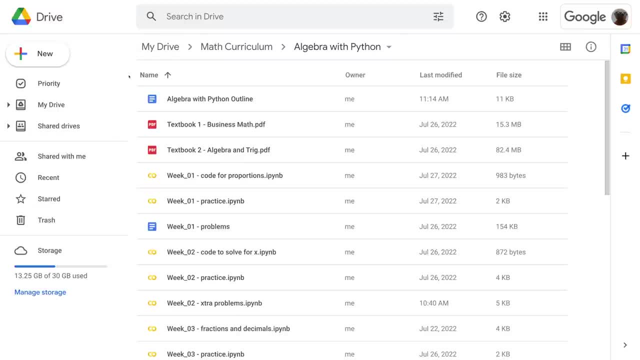 documents and notebooks and everything there, just like, just like I have here And you, you will have access to all these documents. you see, you know soon enough. So if we take a look at the little yellow infinity symbol, that's the Google Colab And 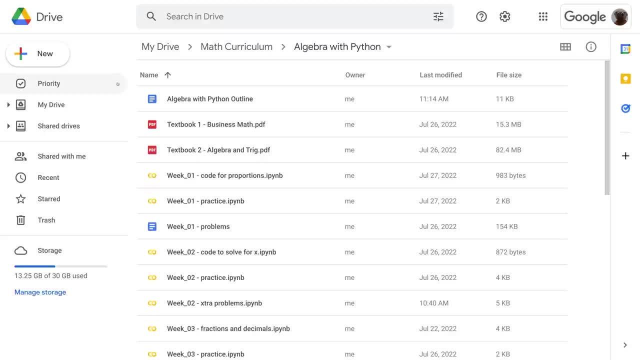 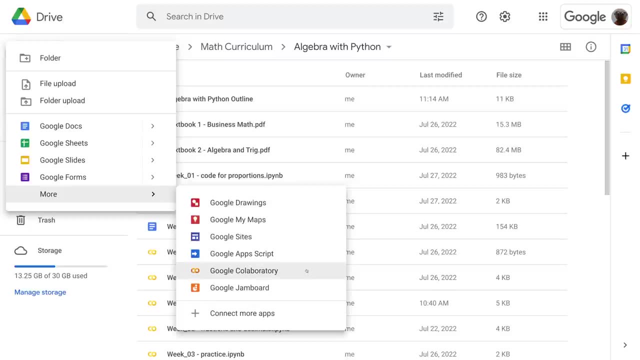 you know, if you want to create a new Google Colab, you're in the folder where you want it to be, click on new and it won't be here and you go to more and then it'll be down here. So Google Colab. 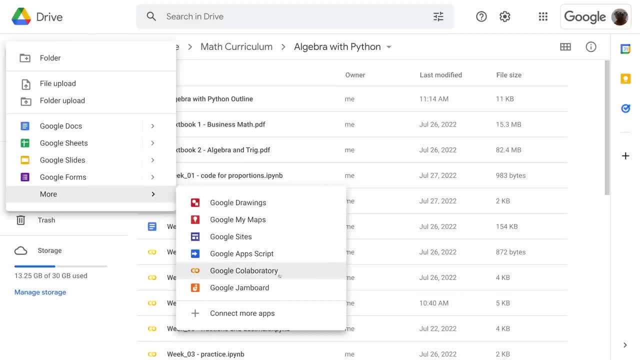 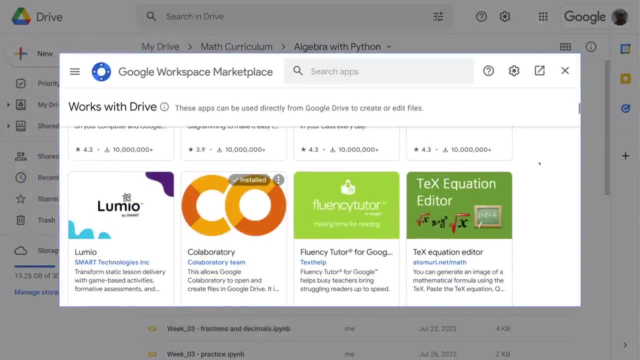 laboratory. Now, if you don't have it already, if you have not yet set it up, then you go down to connect more apps And you know it's. it's begins with C. it might show up, you know, here, but if not, then you can search, you know, look at this like Colab. Even if you don't have it already, you can search, you know, and look at this like Colab. 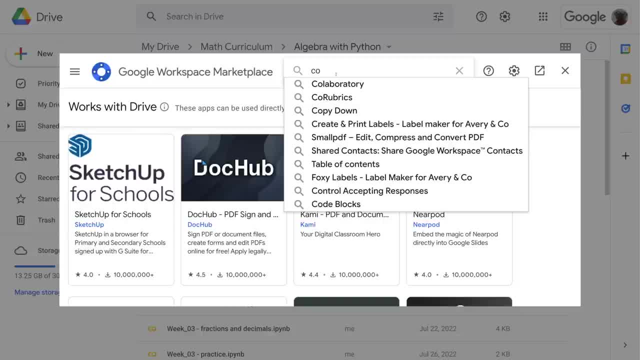 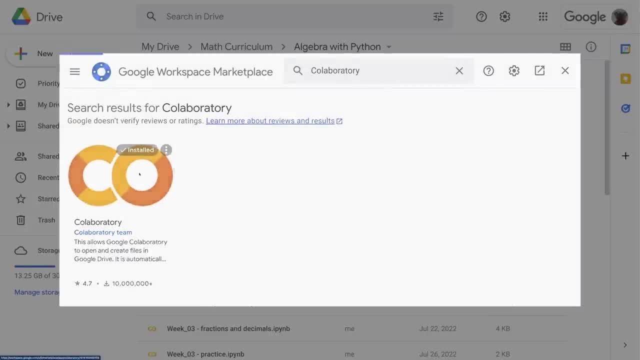 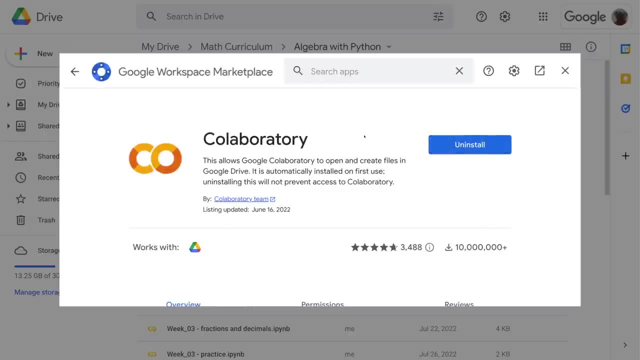 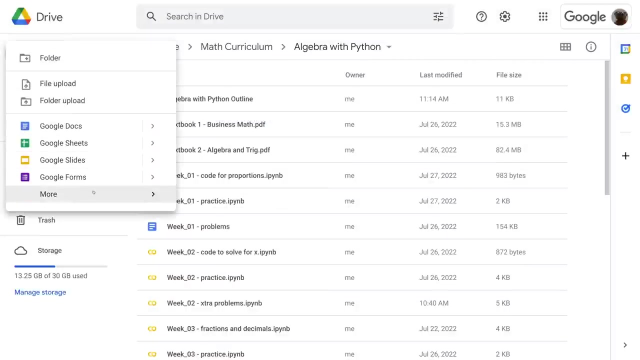 just do co, it comes up. but if you type in Co lab, then it'll come up, There we go. And again, mine's already installed, But if it wasn't, you'd see it there. you click on it And this blue button, instead of saying uninstall, it would say install, and then you'd have have it available. And there we go. Then when you go to new, and then you can go to Google Colab laboratory and it loads. 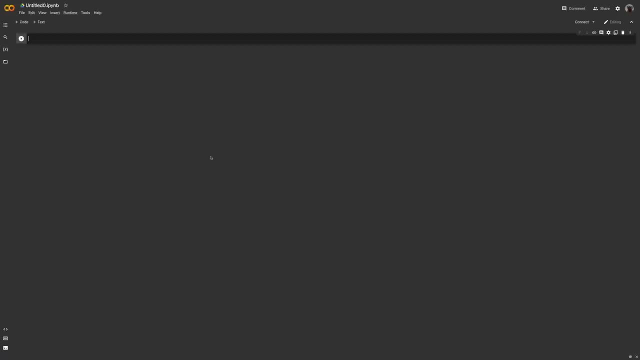 There we go, you go. so, as you see, I like the dark theme for Colab, so that's just the one. that's just what I picked you. you know you can change that. so this little block here, this is where you're gonna write the code. you know it's set up to write a. 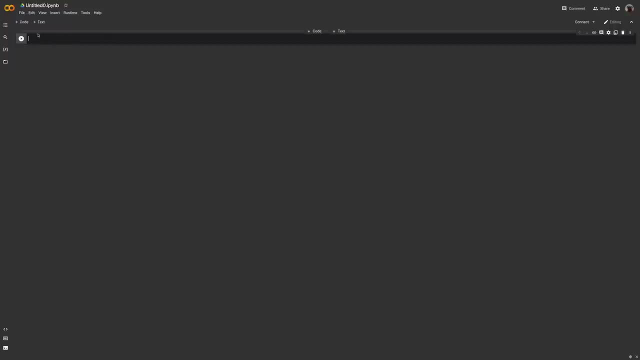 block of code and in addition to that you have the ability to add more code or more text. so you see, you can add another block of code, you can add more text and if you click up there it just adds it in line and you know if you type text now. 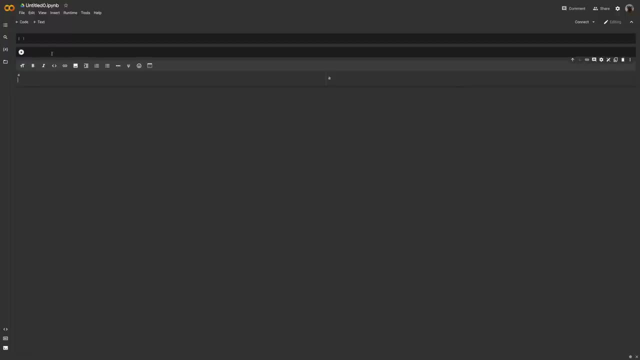 if I hit enter, that just gives me a new line. I have to click somewhere else to get out of that. so there you go. you can add code or text by doing that. also, if you might notice this up here, if you hover around the middle, you can add code. 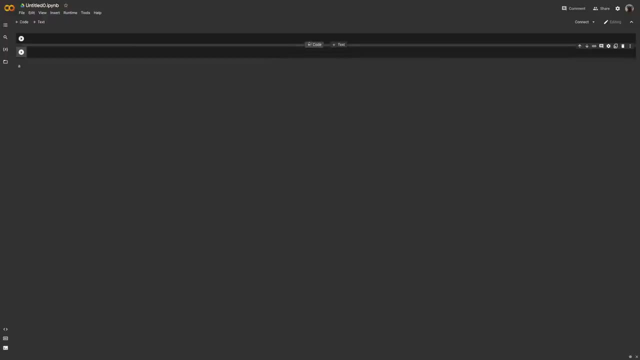 or text, and that works anywhere, you see. so you can add, you know, text right here in between these two, and there we go and that text. actually, besides writing text, you can actually use some, a few HTML tags to, you know, make new line breaks or some things like. 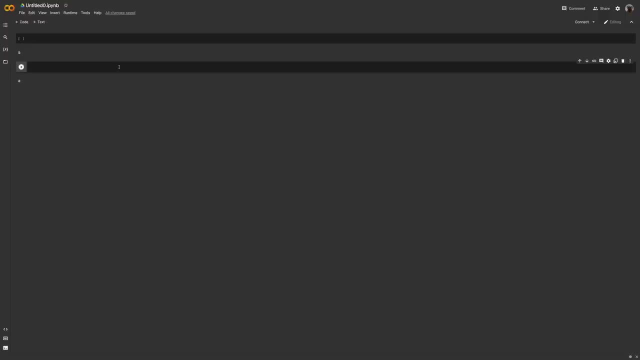 that. and then, if you get really fancy, you can use the latex math notation to display different math formulas. but we'll get to that soon enough. all right, so you have all these different things you can do, your code or text and one of other things you want to do. first, like any document, give it a name and you'll. 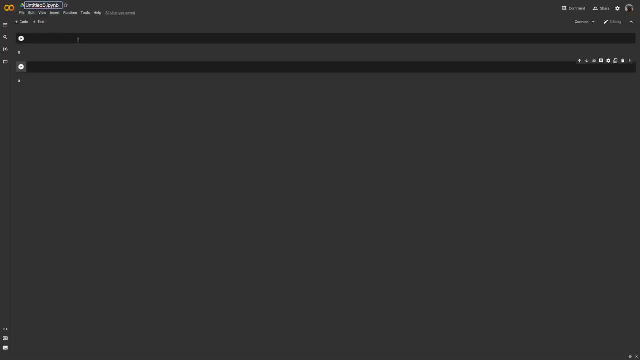 notice the familiar setup compared to other Google Docs. you can, there we go. we'll just call this week one example. all right, so you know, give it a name. you know you don't want to leave all your stuff just untitled. might be, you might forget and it might be hard to find later. and you can write your code there. 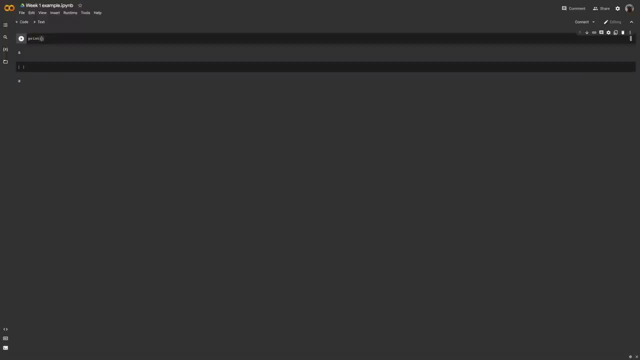 whatever you'd like to put in there, print okay, and you know, there we go. it just sits there as code until you run it and you can click this run button. or if you're familiar with the Jupyter notebooks, you can hit shift, enter. that'll run it also. and there we go. this, this is the output here. notice you can. 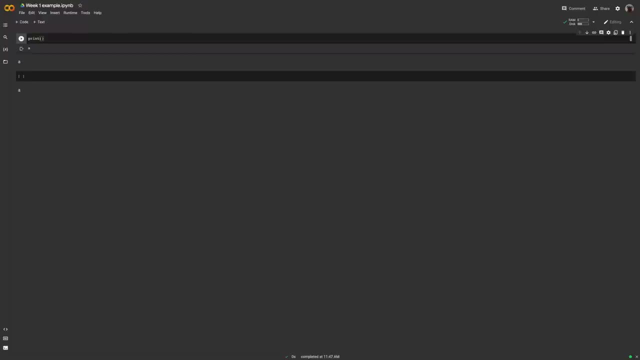 also do a lot of math. you can also do a lot of math right there in the print statement. so if you just put in math formulas, you see, hit, enter, it just gives you a new line. run it you. you can do all sorts of math formulas. and remember the add, subtract, multiply, divide, that all works, that's. 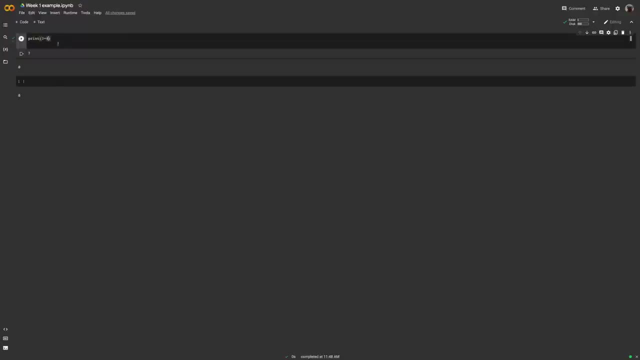 built in the, the exponent would be the. you know, you've got all these numbers right there. you can add in their, через this asterisk, two of them. so there you go. so that would be three to the fourth power, and you say it'll. it'll do the math right there, if you wanted to. 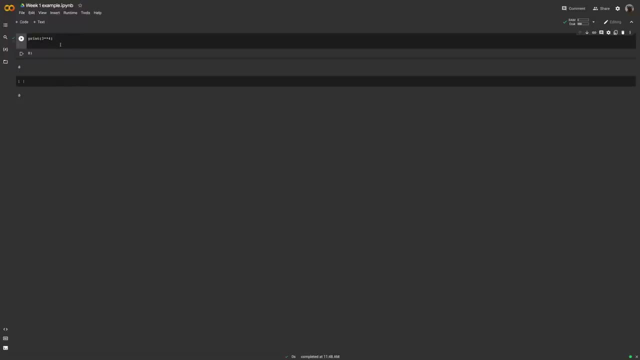 do something like square root. you have to import something and we'll get to imports as we go through a lot of this. but notice, you can. you know you can have your text, you can have do your math for. so for a lot of simple things, you can. 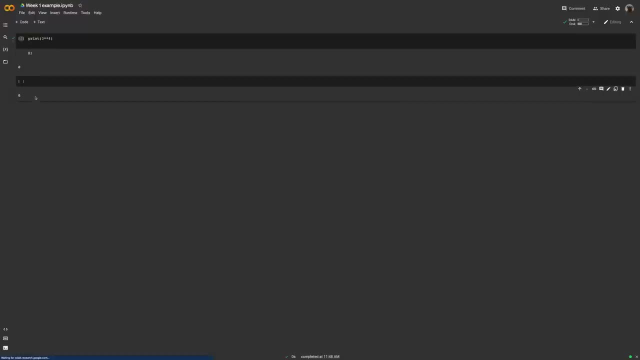 statement. one of the other interesting things you can do is- and if I make this, I'll just make that b for a certain reason- then you have a table of contents here. now, this has nothing, because I don't have any headings or sections, so that's what: the table of contents. 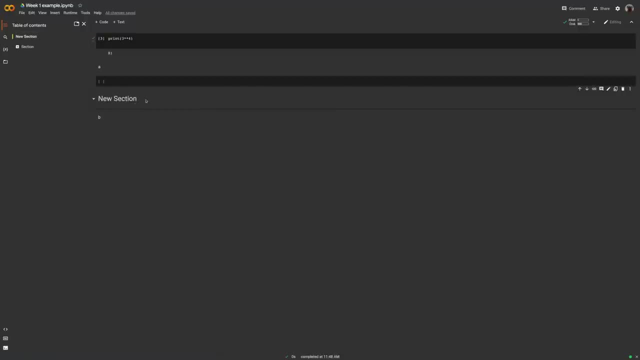 looks for. if you click on a new section, then you can. I'll just leave it as new section and call it right there. you see it shows up in the table of contents and if you double click now, this b is underneath that section. so if I click on this arrow it becomes minimized within that section. 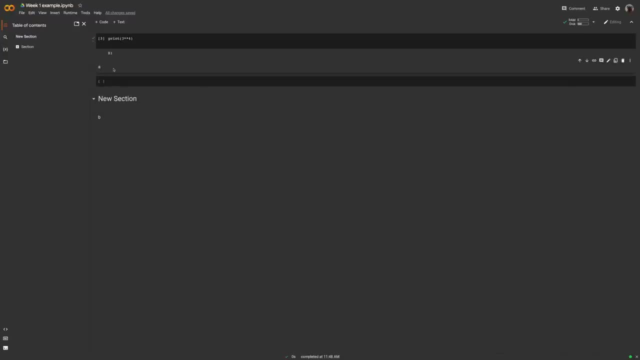 and then here a. if I want to make this its own section, then take a look at the section heading. if I double click on it, it's that hashtag that would be normally used for a python comment. but we're. but we're in the comment. it would be normally. 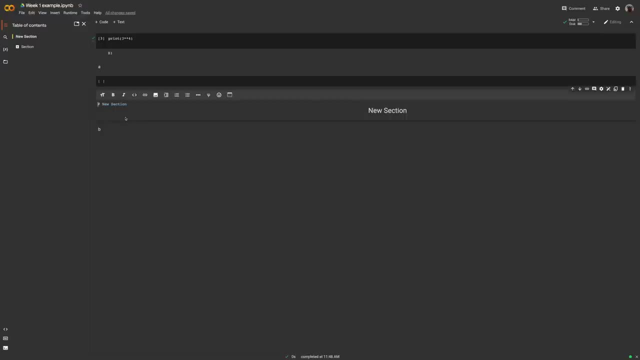 used for a python comment. but since we're in the text part, then you would just use it to indicate a new section. so I can go up to here this text and I can make it a new section. you probably don't need the space, but I like it and again click somewhere else. 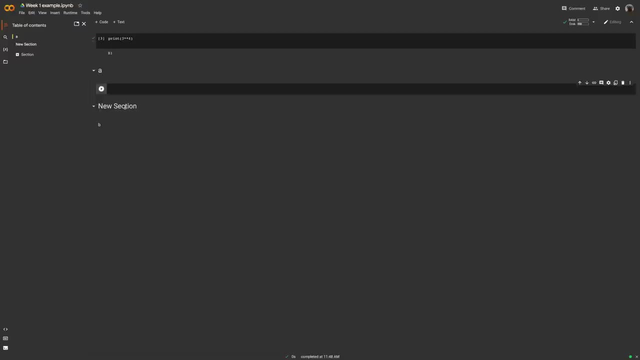 to get out of that. so now I have a and I have my new section here, so I can do some different things. I can put some. I can put some code here and I can in this code I can move it up. see the arrow over there. I can move it up and then maybe I'll make b double click on this and maybe I'll make b its own. 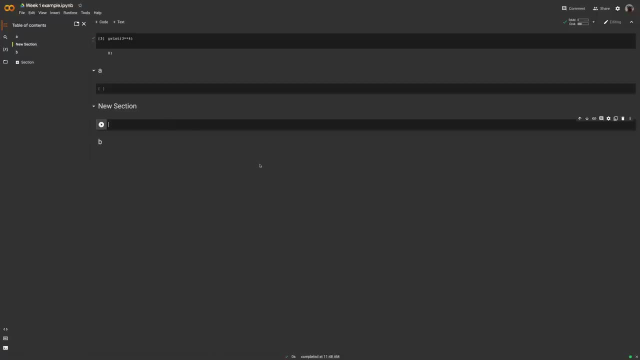 grind, and so I've had someции. now all this click somewhere else, hope that I can irregularizate and so I can have All these sections. now. b is its own section. that kind United, didn't matter, because I don't have anything underneath it. I'll, there we go. 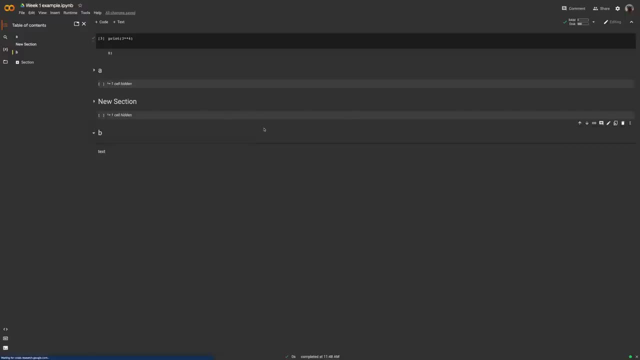 text in here, click somewhere else and uh can collapse it. so you see, I can have these different sections cut clouds and then they all show up in tables content a new section I just fit together. I'd gonna quick classic um deselect. you know apps B. so if you give them names more than A and B, it becomes useful because you can. 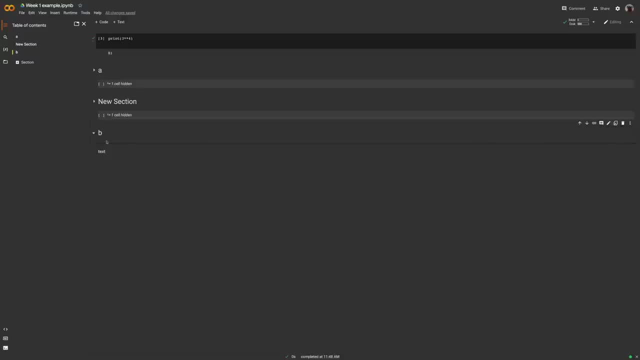 find them in the table of contents and then you just click to expand each section in whatever else and you can have within the section. you can have code text, you know, and as many of those blocks as you want and that section goes until you create a new section. so some good, useful things you can do in. 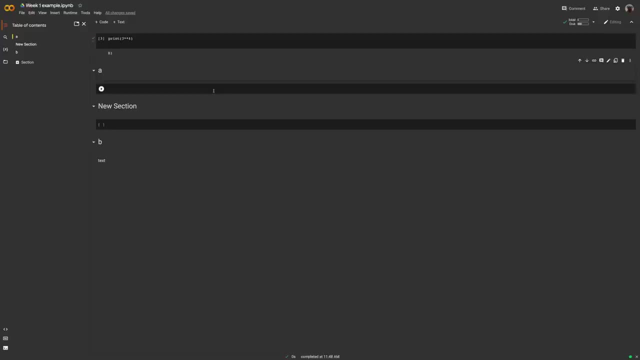 building your own Google Colab notebooks. you might decide that that you might like that as an organ to see as a way to organize them. you know, keep them in sections, so that helps also. the Google Colab like a little everything else in the Google Drive. it does save automatically, but it doesn't do it as 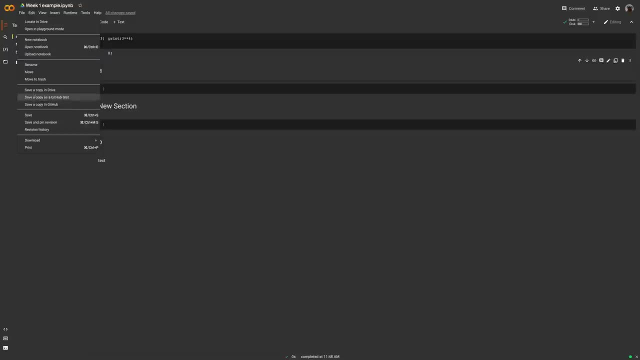 often. so you do have a file and you do have a save here and also the normal shortcuts, ctrl s or command s. so you that that does work and that way sometimes you know if it goes a while in between saving. if you try to close it it might actually prompt you to say that you might need to save. 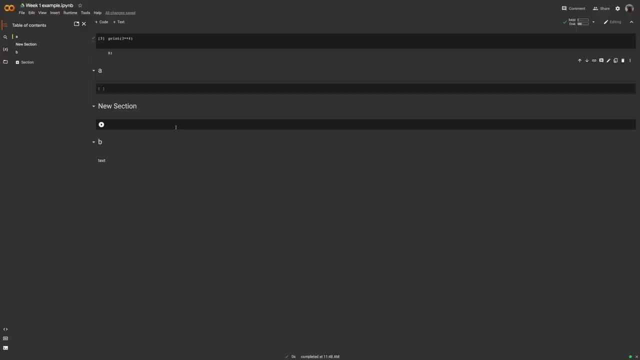 it. so that's just something to think about. that you know you actually do say you do actually make an effort to save things here in the in the Google Colab. so we set up our code. we can do math right there in the print statement. we set up our sections table. 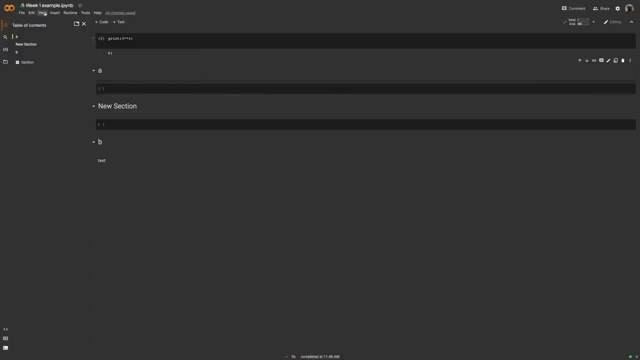 of contents and all these sections. you know, within the view you can actually expand or collapse them all at once if you want. you know that's kind of interesting and through all the code we're going to work on, you know you also have down here one of the other things. it looks like you know xml or HTML tags in that list over here. I've actually got, you know, lab sandals on my first computer interface palette, so you can kind of look at the library suites, trouver contextual information with the same software things that you could afford you know. next you can look at the desktop software. 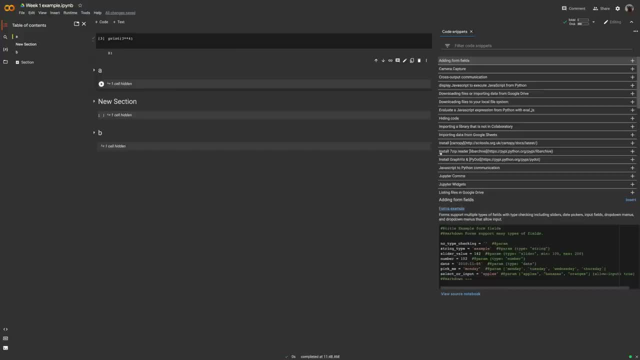 PSPplaces here and you've got some inspection on another of those things or the setup teams and so things around doing things here. you know things up a tags and it's a bunch of code snippets that you can use. you know copy and paste. try these right. 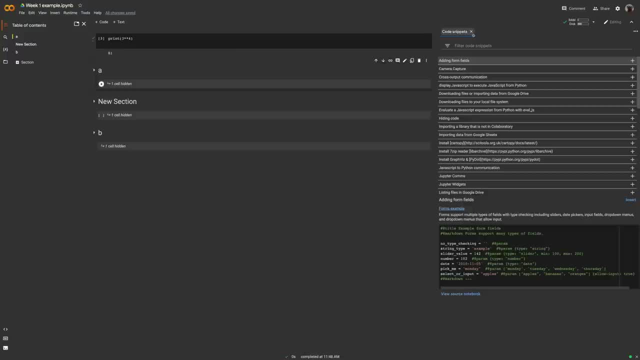 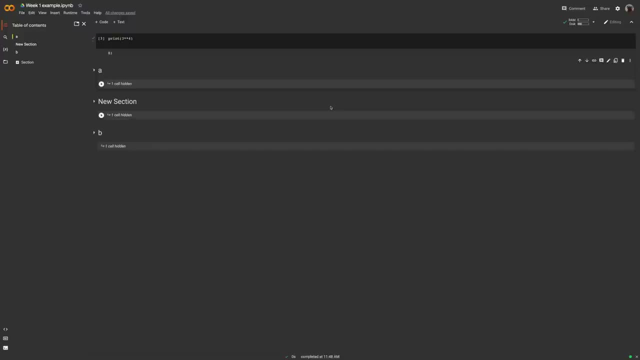 in your right, in your google collab, right here. so some pretty cool things to explore. and there we have it. um, you're going to be building your google collab notebooks. um, you might, you might want to build one for algebra and you know, just continually add to it in this. 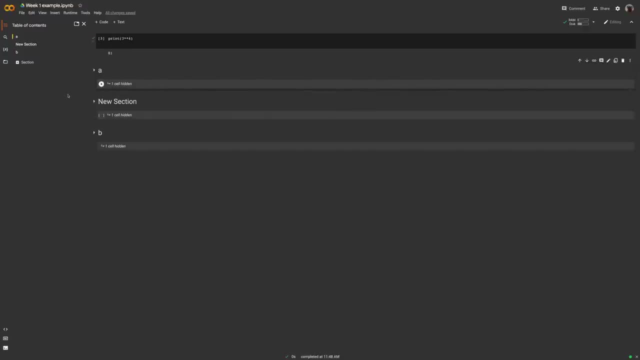 case, definitely make sections, because that's going to be helpful table of contents to find what you want. so you could do that. you could make a different notebook, you know, for each unit or each week, or however you want to organize it, but then the idea is you're building these resources. 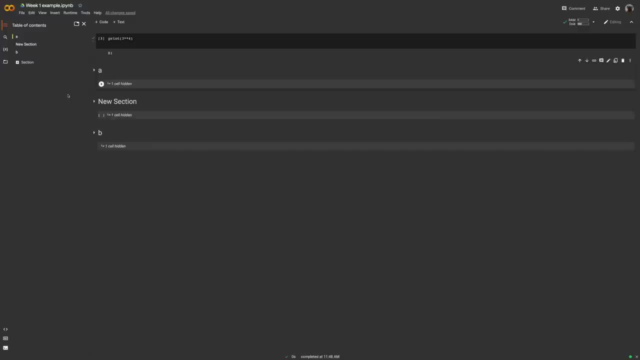 that you will have access to and, as well as installing it on the google drive, you can also download and install the app, so that'll be useful. have it on your phone that, when you first run it, you need to do a couple of things. you need to do a couple of things. you need to do a couple of. 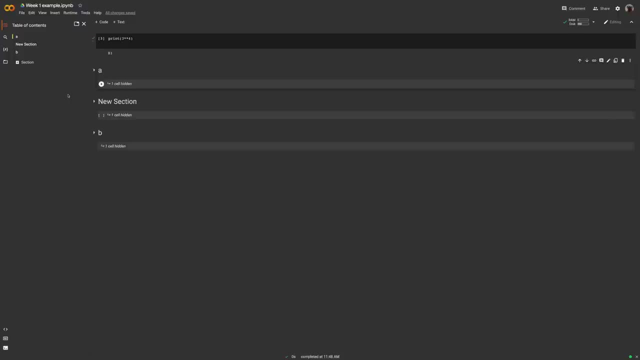 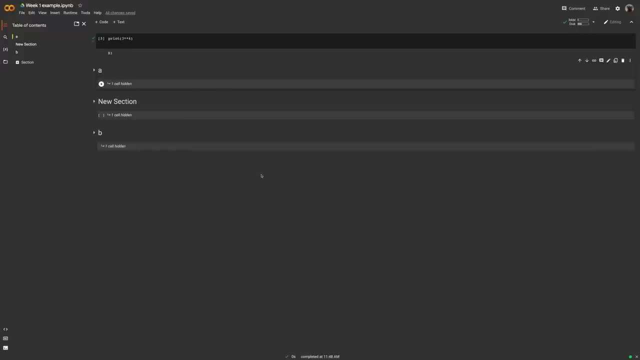 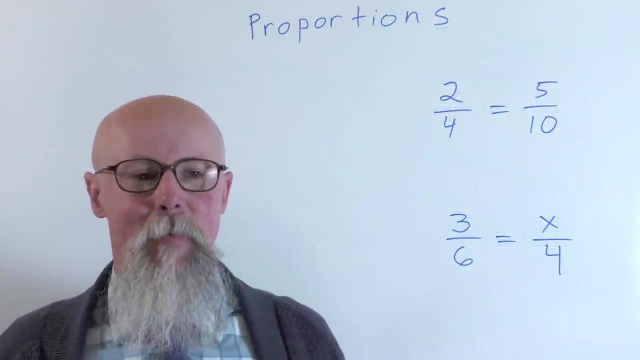 your Google, in your Google CoLab, And it's going to be exciting. we'll get to a lot of, a lot of interesting things. So let's, let's get into the math next. So we can't talk about proportions without talking about ratios, And a ratio is another. 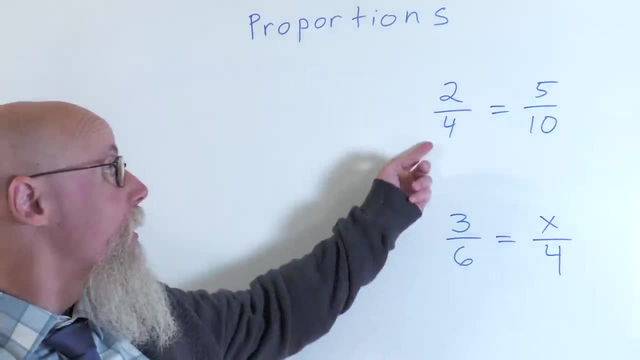 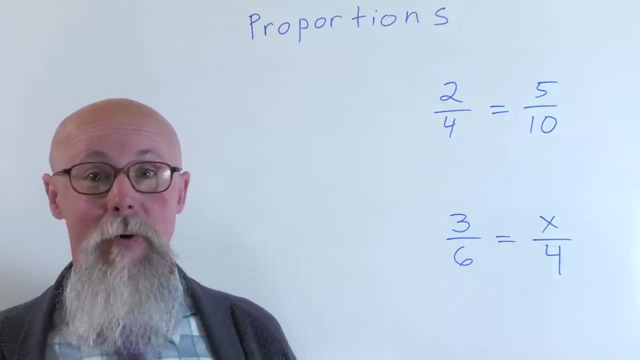 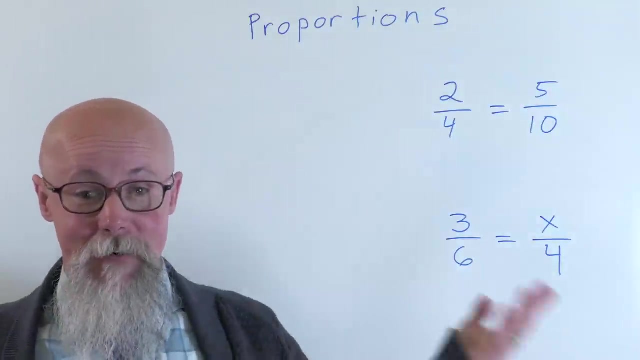 word for a fraction. So this: two out of four- I can write that as well, two out of four, but I could say two fourths. I can call it a fraction, but it's also a ratio, And then a proportion is two equal ratios. So if I know that these are equal, then there's other things I can. 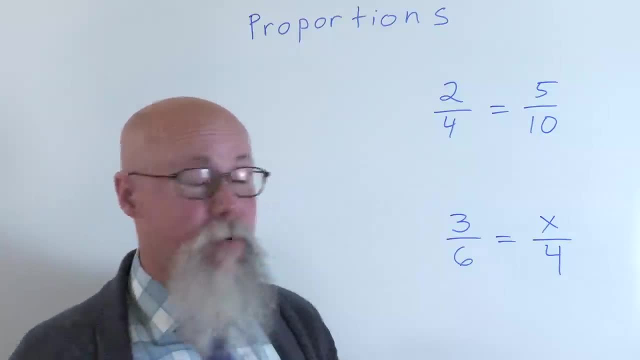 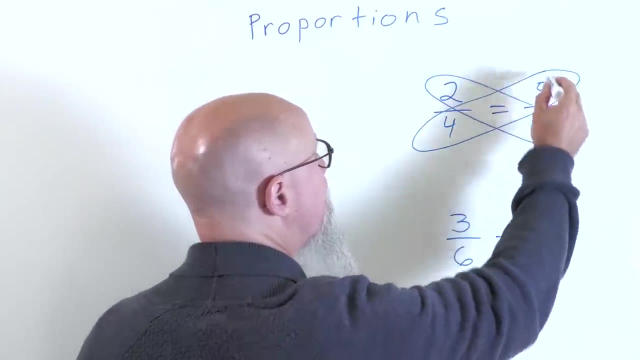 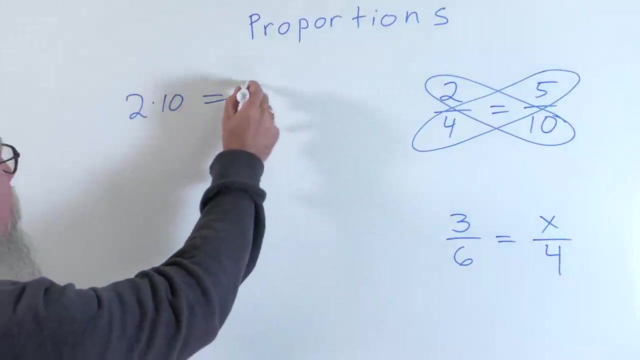 do with this, And one of the things that works and becomes very useful is cross multiply. So if these two are equal ratios, then I can cross multiply. multiply the diagonals, I can do two times 10, equals four times five. 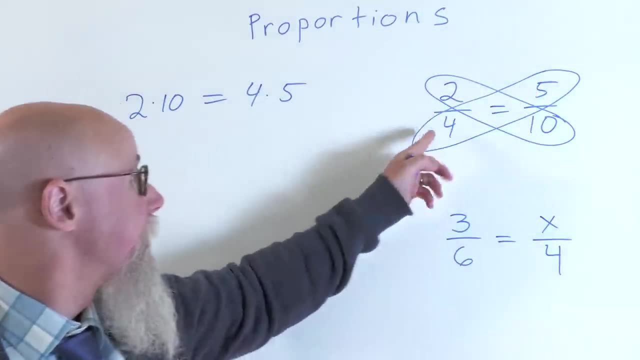 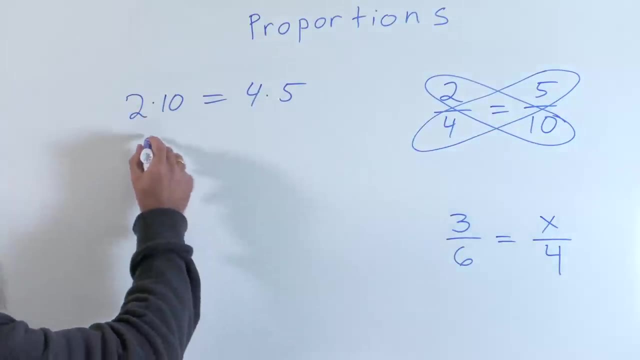 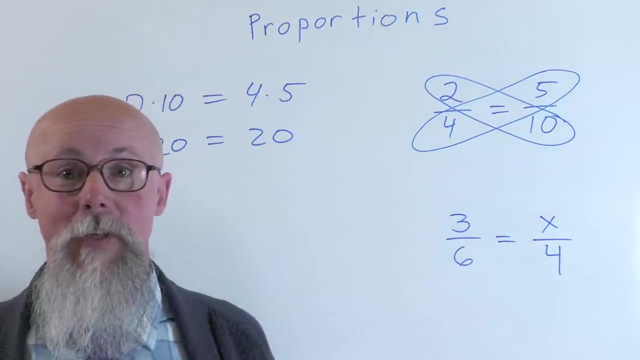 And that's another way to write this. So then I can get it out of the proportion mode And I can use this to double check or I can solve for things. So two times 10, we see 20 equals 20. And then that's true. So you know, we confirm that that works. we can always do this. 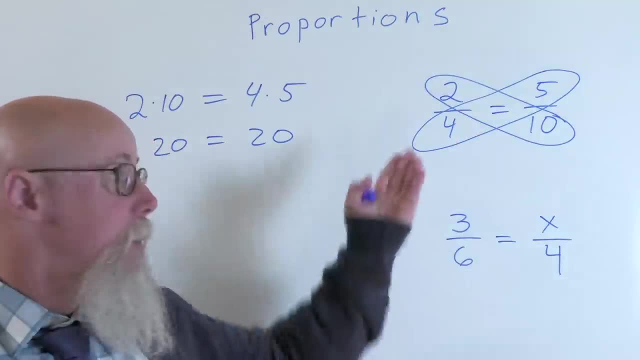 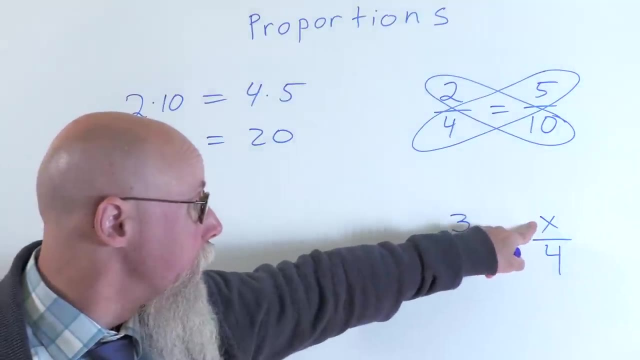 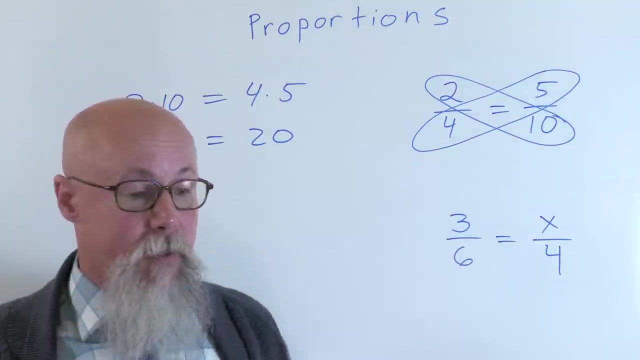 If these were other numbers, I can check to see if this really is true, cross multiplying, because if that doesn't work, then that wouldn't be true, And I can also use it if one of these numbers is unknown. So if I have three out of six equals x out of four. Now there's other. 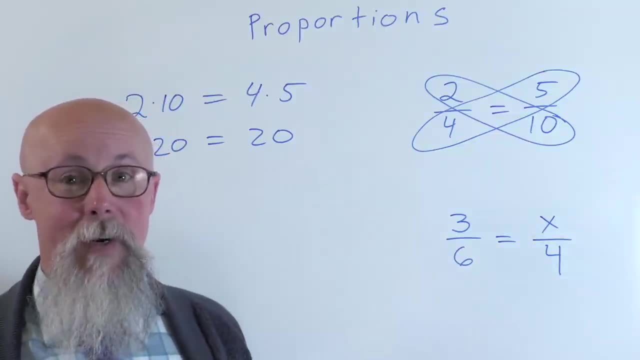 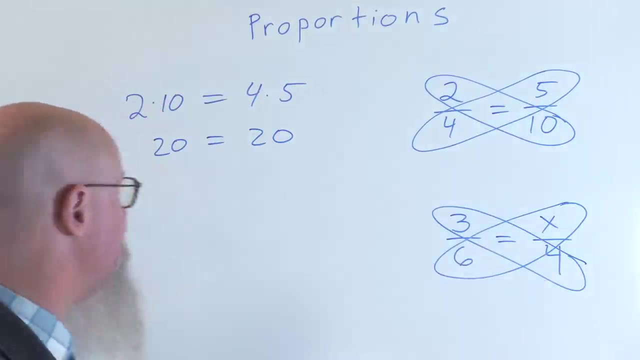 ways to solve this, But this is the go to way because it works every time. So when I do this, I do my cross multiplying. Then I can do this: three times four is 12 equals six x. So there we go: Three times four is 12.. And then six times x is six x. And then I know that the next step I'm 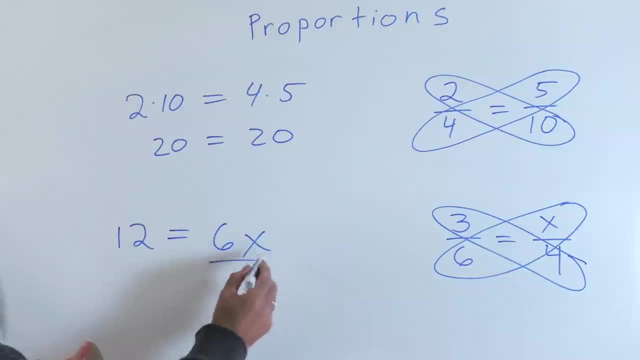 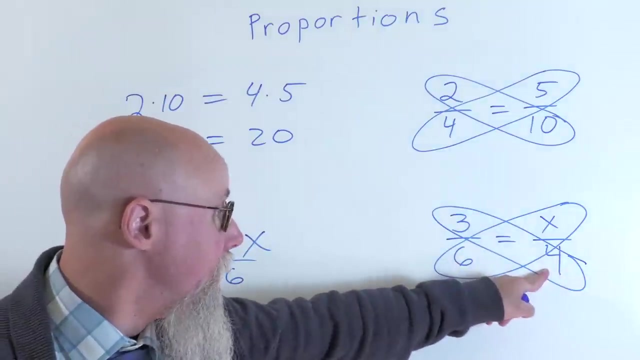 going to do is going to be dividing by six. So then I get that x equals two. Now, doing that, we can jump ahead and say, okay, let's. I know that when I multiply this diagonal, I can picture this step: it's going to be six x. So the next thing I'm doing is dividing by six. 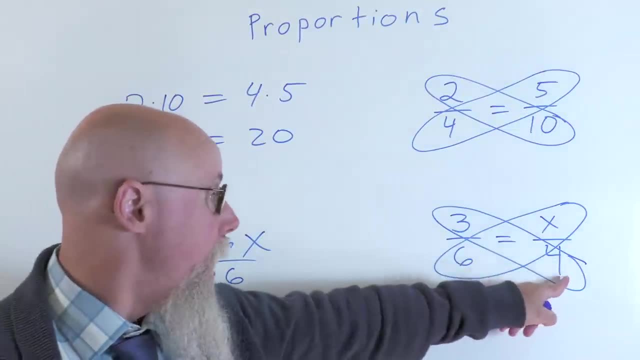 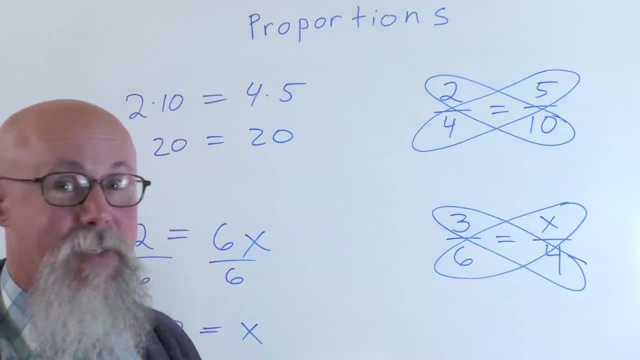 So a lot of times we just put this in one step. So I multiply the diagonal that I can divide by the other number, because I know that the next step and then my answer is x. So we can really make use of this in in writing code. I can see the proportion. 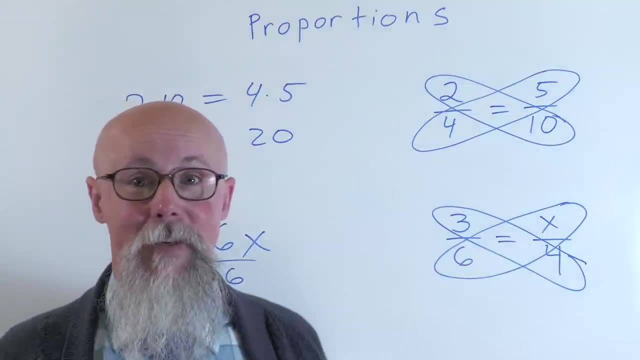 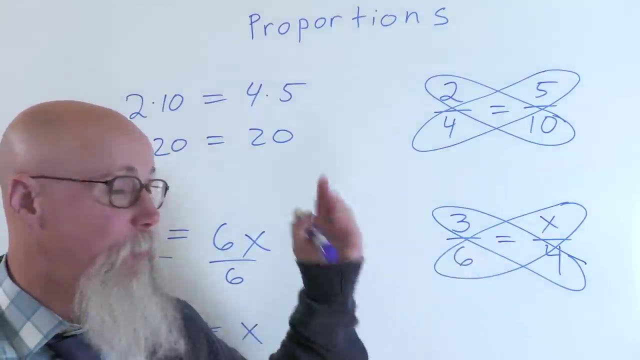 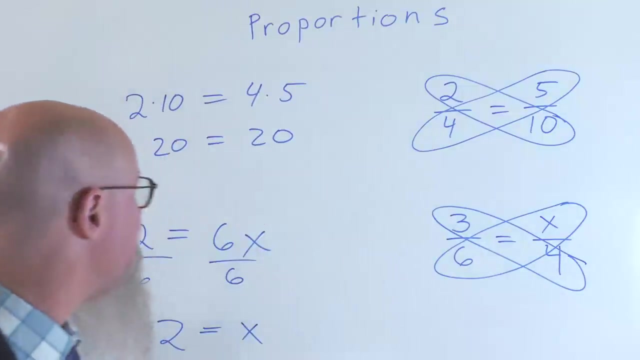 and I can then just put this on one step to solve for x. And again, that's. it's the go to way it works every time. So I can write code to then prompt for these numbers cross, multiply and then solve for x. One of the ways this is also useful is some of the other applications. If I 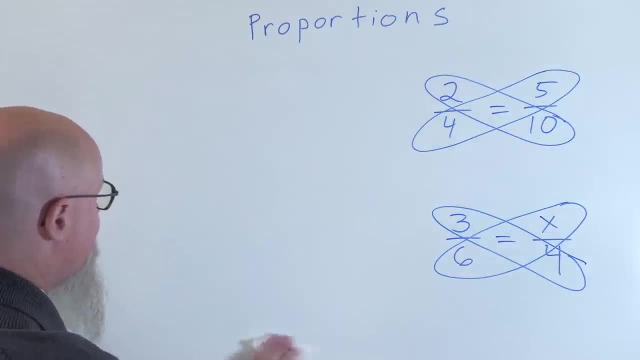 have. let's say, I'm converting something like miles to kilometers. So if I have you know one, is you know about 1.6 kilometers, then I can set this up. this is the ratio that I know, So as long. 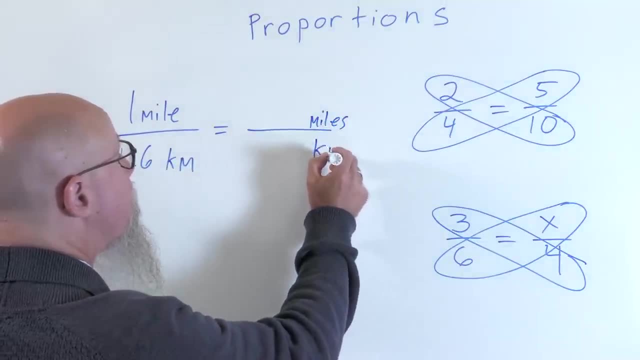 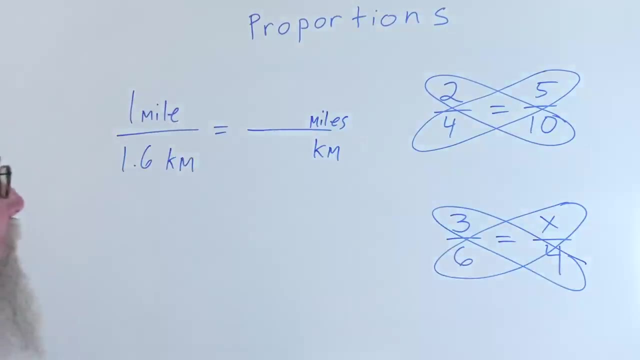 as I have miles and then kilometers, then if I know one I can figure out the other. this unknown can be either place. So you know, if I have, you know, two miles, then how many kilometers is that? 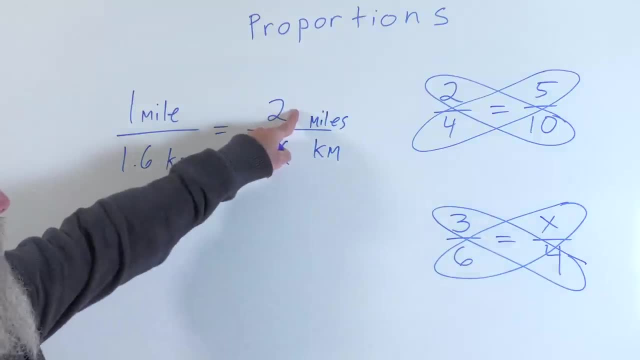 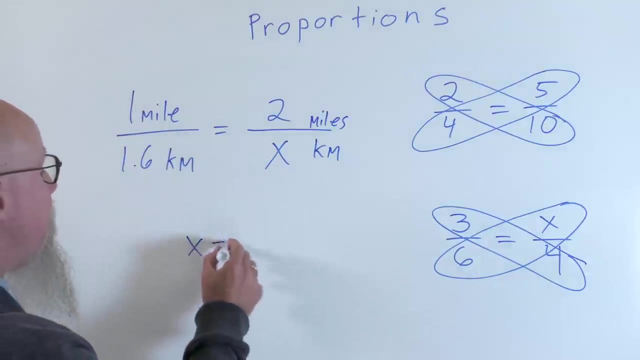 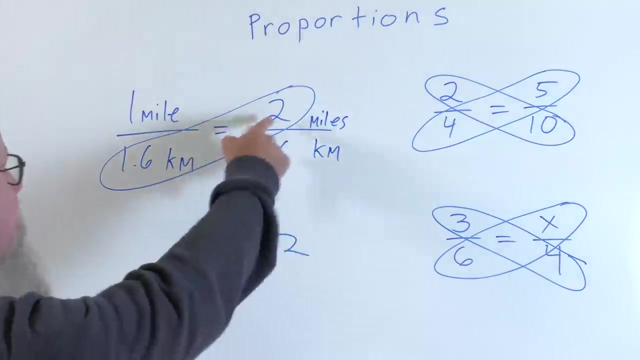 You see, we can make use of this. I know that I'm cross multiplying two times 1.6, divided by one, And then so there we go. So x would be 3.2. And again, I'm multiplying the diagonal that I can two times 1.6, dividing by the other number. 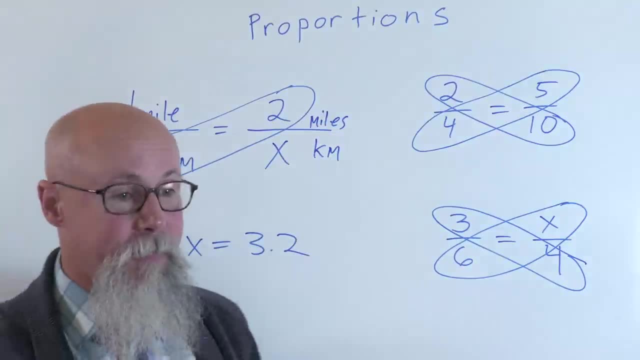 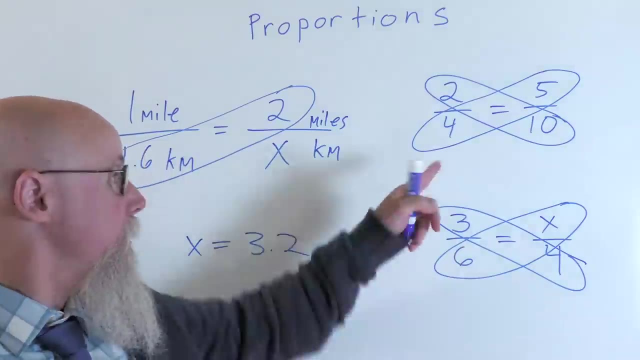 which, in this case, it's convenient that it's one, so then I can solve. So this is what we're going to use And we're going to take a look at how to put this into code. And so prompt for you know these four numbers. 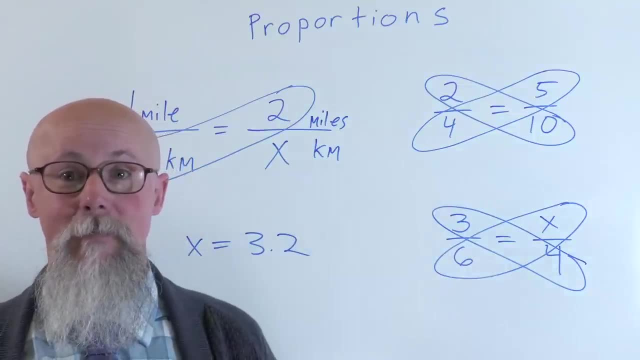 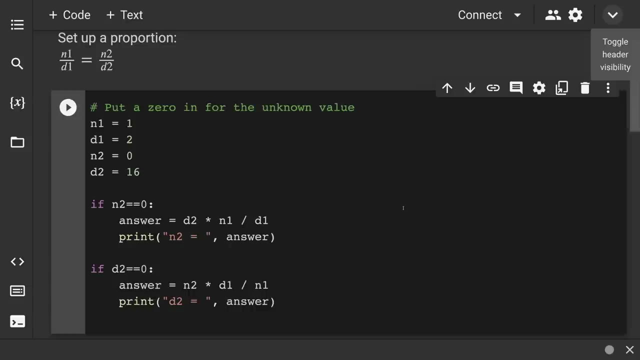 or three of them and then figure out the fourth one. So let's take a look at how that'll happen. So let's take a look at the code. So we're going to see here how much easier it is to write some. 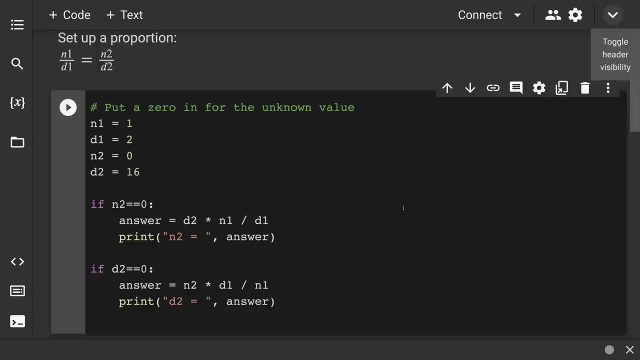 code to solve some of our problems. And, just like proportions, we have that cross multiplying that we know works every time. So I'm going to put just a display here to remind us that we're setting up the proportion, And here's what it looks like. 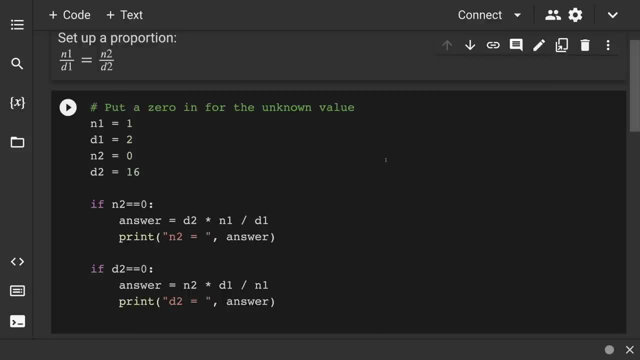 So if I have a proportion, I would know one of the ratios. So I would know, let's say, n1 and d1.. And then n2 or d2, one of those I would not know, but I would know the other one. So I have my. 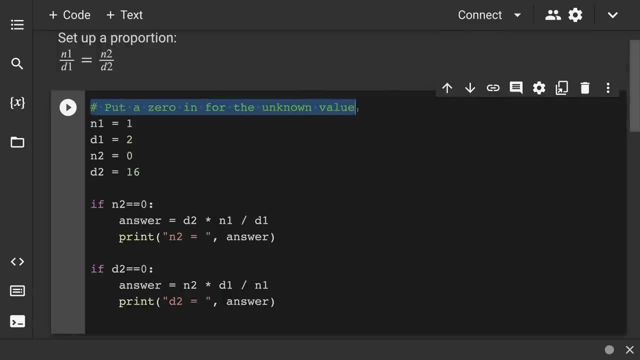 comment: here in the code, put a zero in for the unknown value, because realistically none of these values would be zero. That would just you know, you wouldn't even need to think hard about that. that zeroes everything out, or if it's in the denominator, it's undefined. So that would never occur in something that we're. 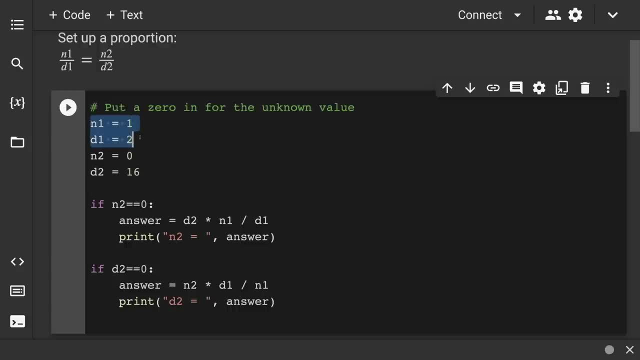 really trying to solve. So I would know n1 and d1, and I would just change these numbers, put in my numbers that I know and I'll put a zero in for the one I don't know, And then I'll put two. 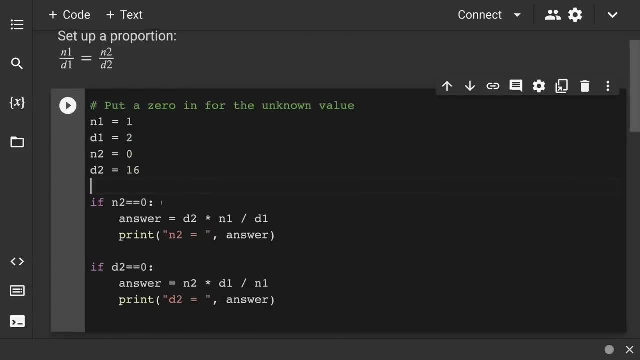 if statements. So I have if n2 equals zero. and there we go. Notice the setup of the if statement in Python: If n2, the double equals, because I'm testing it- I have a colon And then the indentation afterward is one. 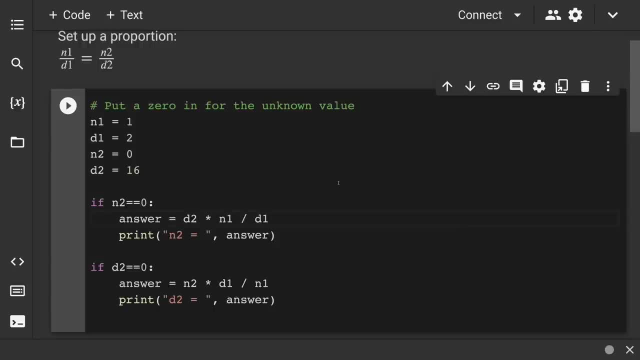 two, three, four spaces. I would hesitate. some people use a tab. I would hesitate to not use a tab. They don't often give you the right number of spaces. So indent four spaces and then I would have. the answer is- and I'm going to just do that- cross multiplying. So you see d2 times n1, divided by. 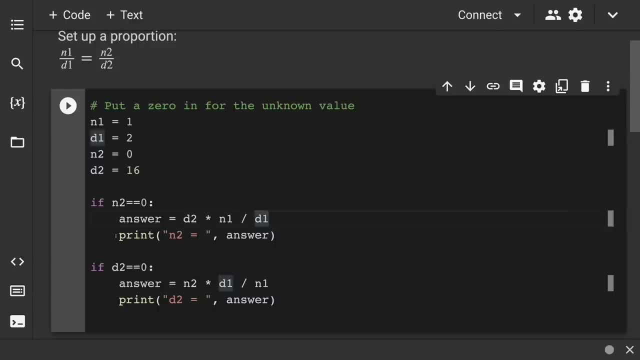 d1, that cross multiplying. that we know, and then we'll print out the answer And we'll do the same thing here. if it's d2, that I don't know. So my if statement: if d2 equals zero, colon, four spaces. 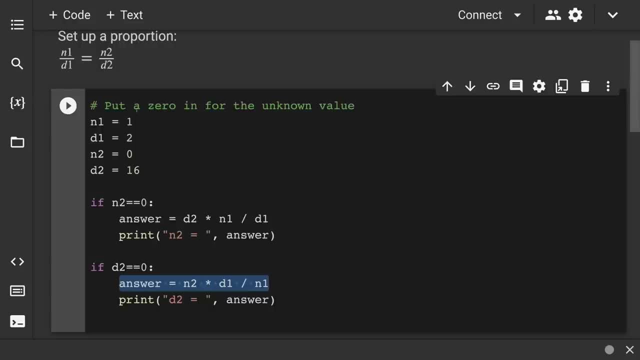 indent and then this answer: Notice the cross multiplying. So d2 is what I don't know. So I'd be doing n2 times d1, divided by n1.. And then I'd print out that answer. So there we go, And then, given these one over two equals, what over? 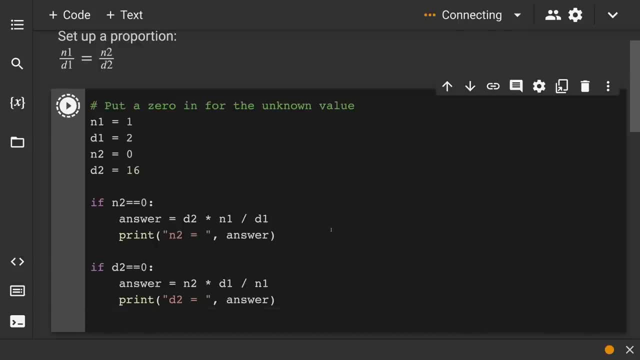 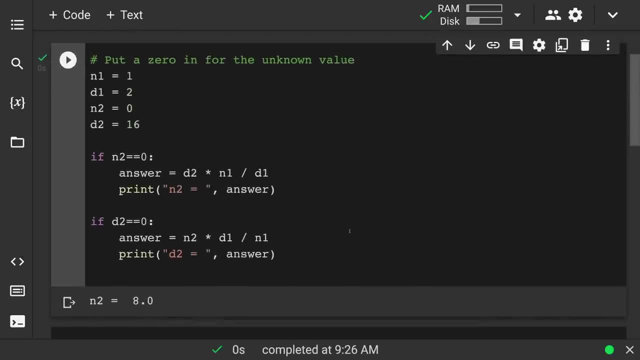 16.. And then if I would run this and it will output the answer right here, There we go. And two equals eight. Or if I had this, I'll keep this and maybe I'll put this: one is zero Rio. and if we run it, there we go, Really. 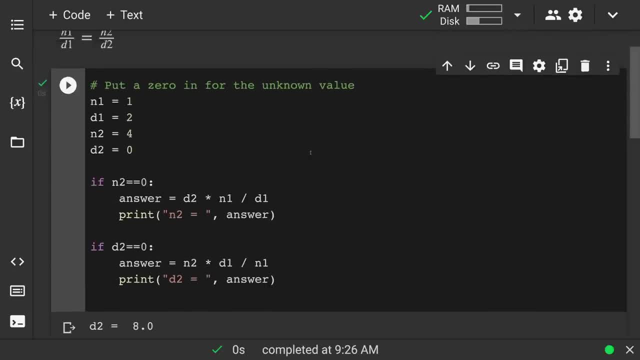 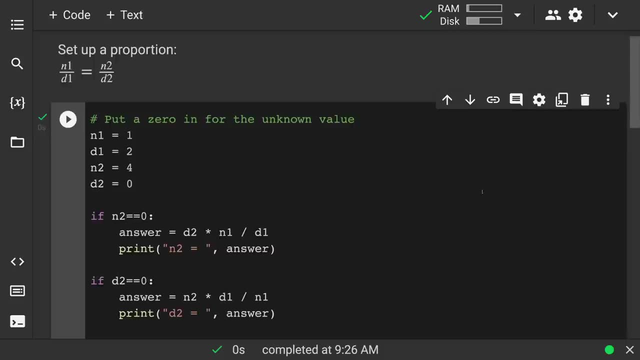 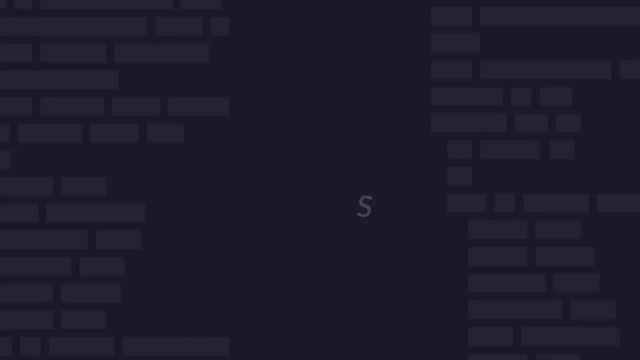 straightforward. We want to get to this point that we know these, we know these formulas and we can just put something in here, maybe even display something to set it up, and cross, multiply, solve any proportion this way. Now that we've worked through the 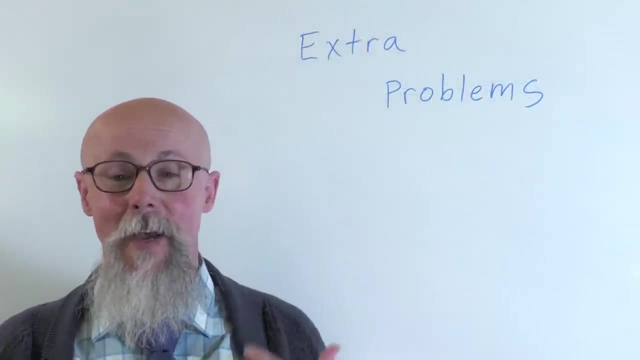 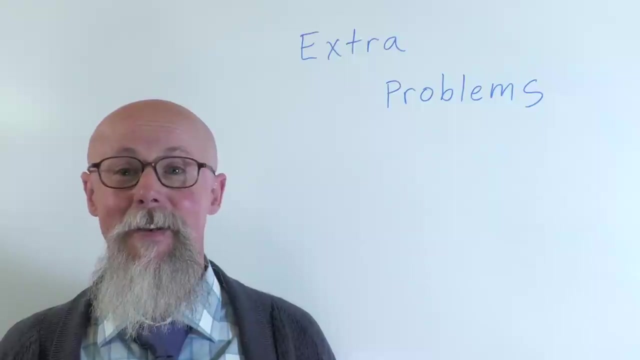 four skills in this unit. let's look through some extra problems, And I'm going to work through extra problems using the Colab notebook So you can see how you can apply these resources that you're building and use the use these to solve problems that might come up in a textbook or in. 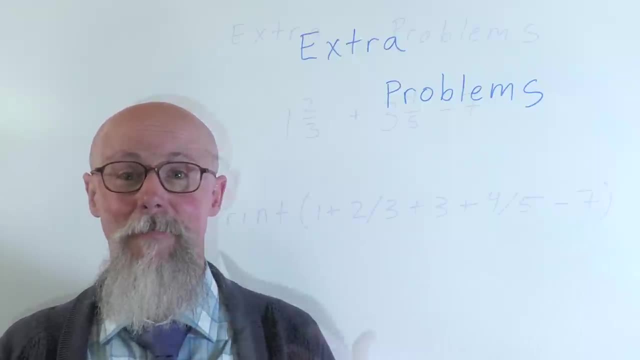 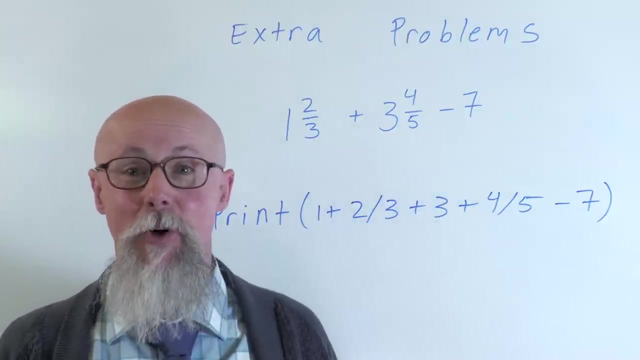 day to day life. So we're going to go through some more extra problems here. We're going to work through some extra problems here relating to some things that might come up in working with proportions, ratios and one of the things that comes up. you know, we work with mixed numbers And in math I 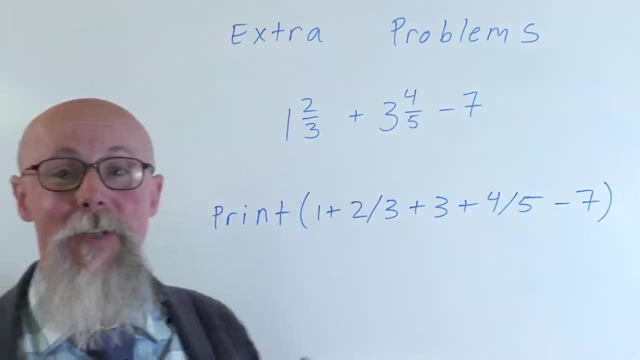 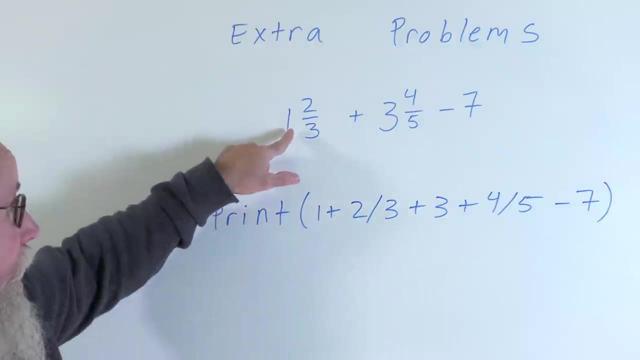 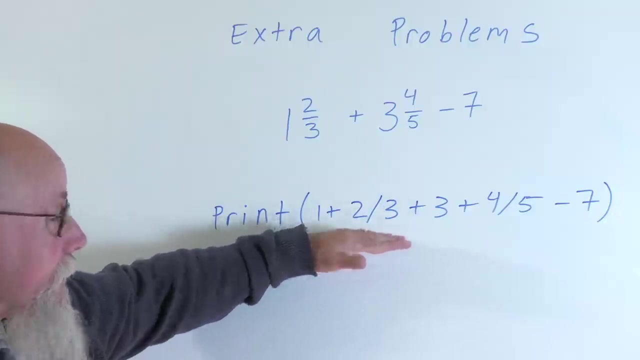 might write it like this. But then you think: how could I do this in Python? And Python, remember, you can even do math in the print statement. So you could put this as one and two thirds becomes one plus two thirds And you see two divided by three. Notice, I didn't even. sometimes I use 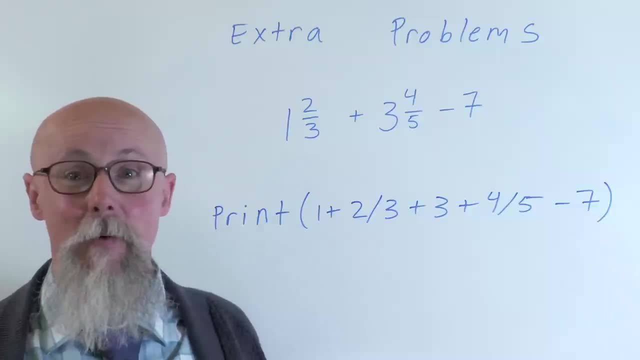 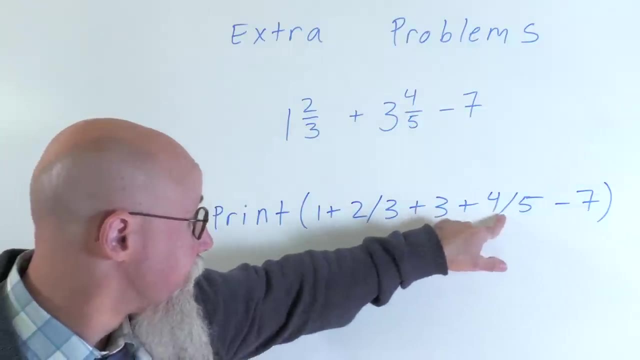 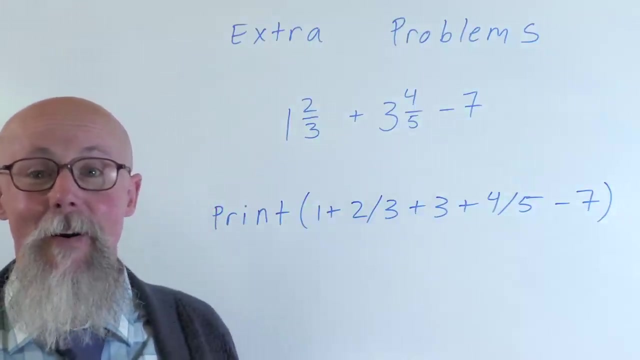 parentheses, extra parentheses. But we really don't. Python knows order of operations. So you can have one plus two-thirds, plus three and four-fifths. so it would be plus three plus four divided by five, and you know you can change it up, minus seven. you can put that all in a print statement there. 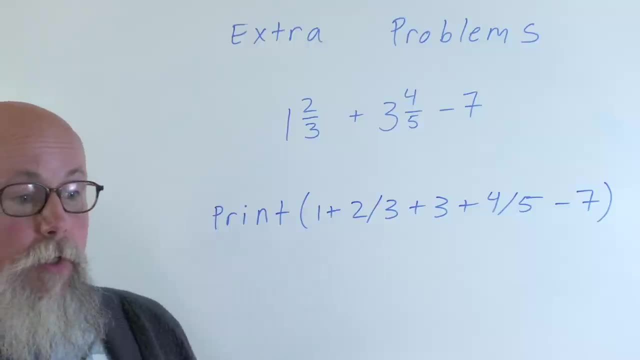 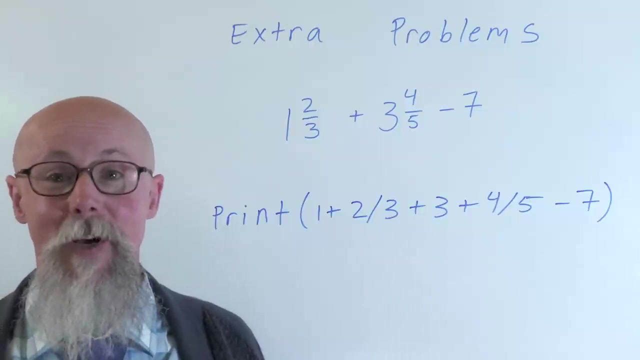 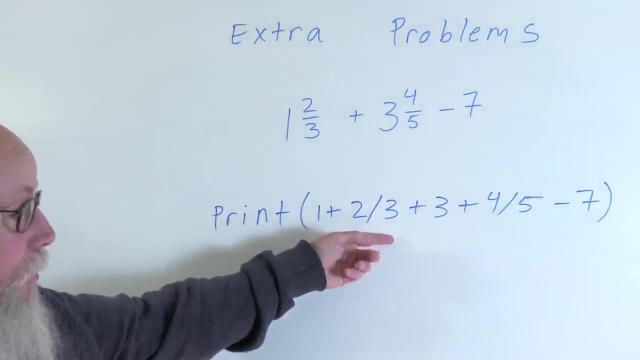 and it would output the answer. now, later on in, i think, the third unit, we're going to also talk about converting that output- if it was a weird decimal- into a fraction or mixed number. but we'll get to that. so you, you can do this, but even also at this point, you could if you wanted to. 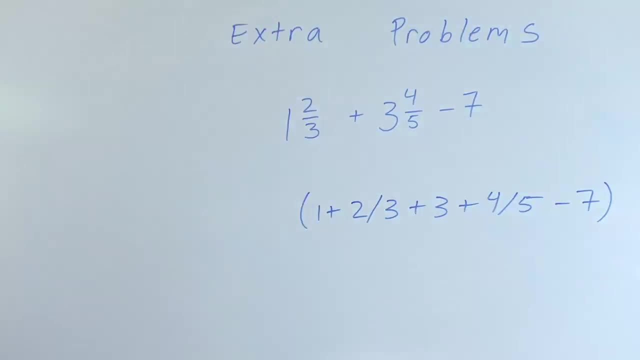 instead of print and you don't need the parentheses, but i i'll just keep them there. you can store them as a variable. so if you had something that you wanted to store as a variable and then use that later on, or any one of these you know, convert a mixed number stored as a variable. 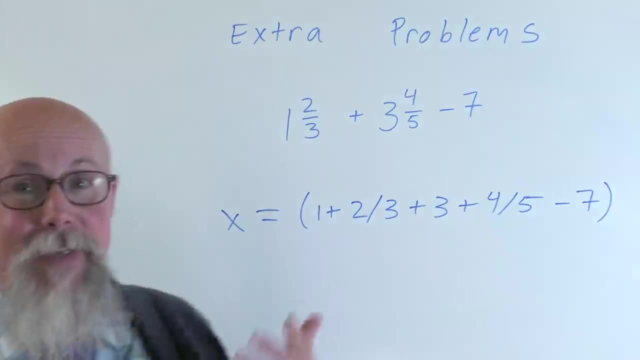 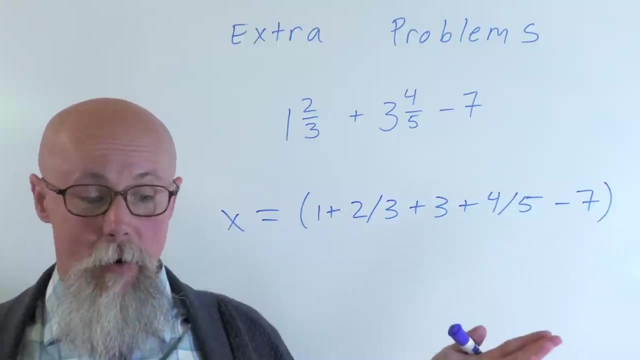 because some of these like two-thirds, that's, that will come out as a mixed number, or the, or one and two-thirds that will come out as that repeating decimal. well, later on you might want to keep as many of those decimal places as possible and storing it as a 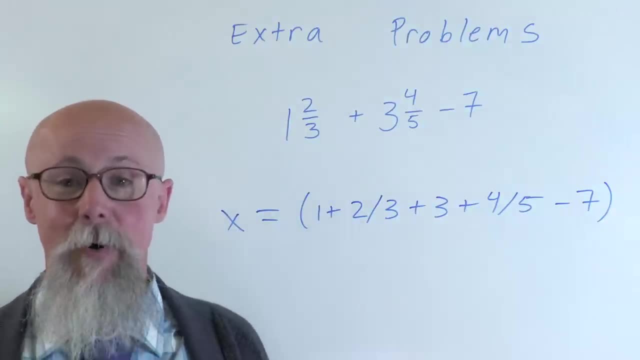 variable will do that for you without you having to write down all the decimals. so really that's the whole thing we're trying to build. you know, for all the different times you might use a calculator, hey, might as well use google colab, because you can have all these formulas in there. store variables. 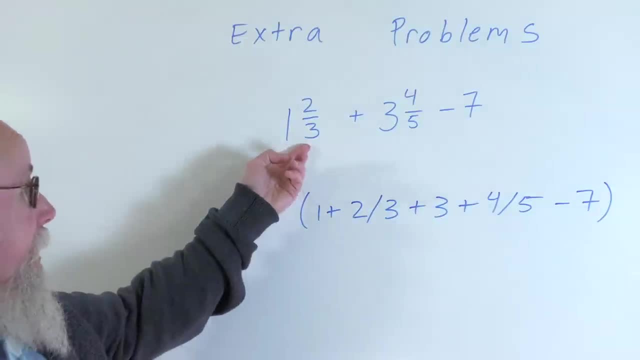 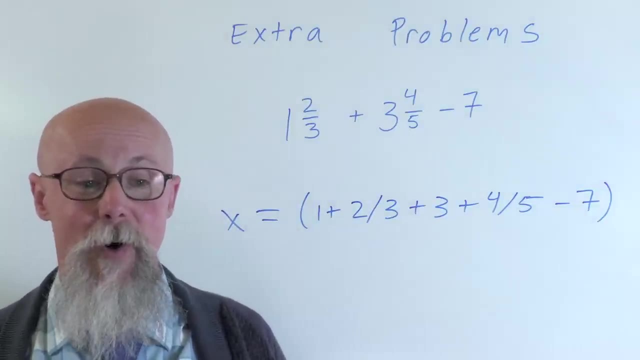 and everything. so for all the different times you might need to work with mixed numbers, yeah, print it out, store it as a variable and continue on and work with the rest of the problem. so if this comes out as a repeating variable, let's. let's take a look at one other thing here. if this comes out, so let's. 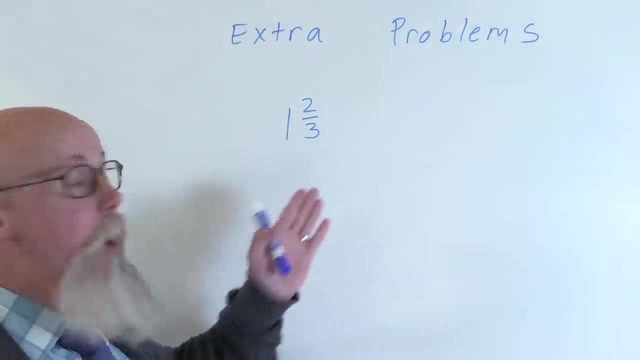 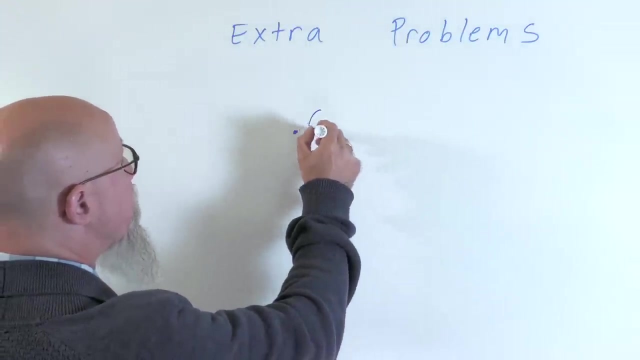 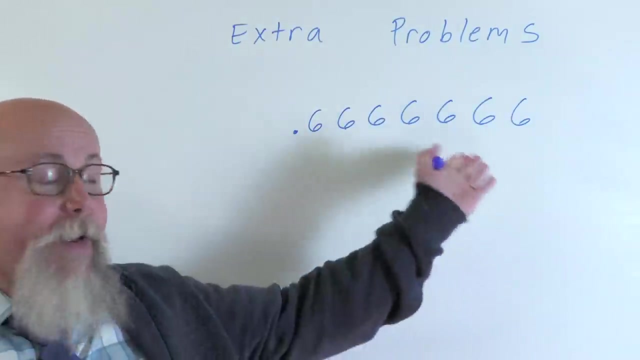 just say i have that, uh, one and two-thirds. so we know the one, but if i look at the two-thirds, you know that would be, you know, 0.6 and it keeps repeating. you know it'll keep repeating. if you get output like this, how would you know that that would be two-thirds? well, one of the ways 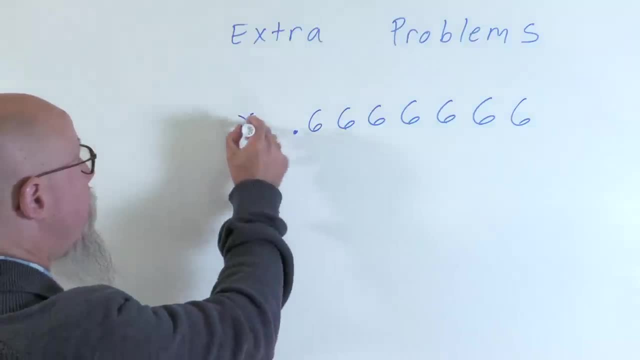 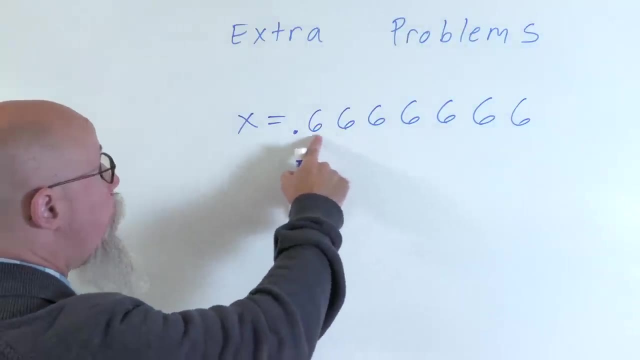 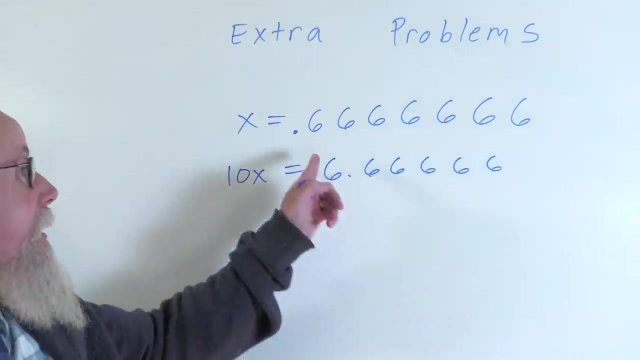 you can do. this is: we can throw in some other variables here. let's call, let's call this x, so x is all these repeating decimals. so if it repeats each um, each place, then i just need to multiply it by 10.. you see, and that keeps going, because if this keeps going, and then this keeps going. 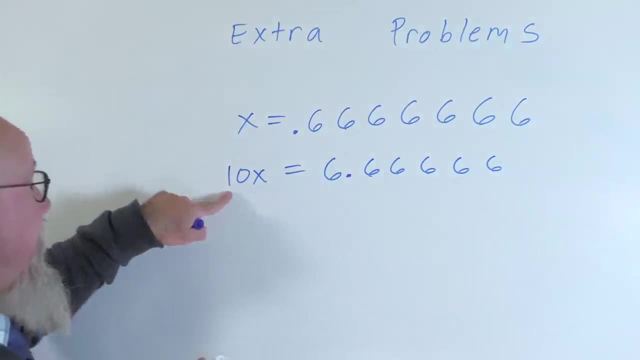 then if i subtract them, 10x minus 1x, so that would be 9x equals 6.. now notice, i did not rewrite it, but i am subtracting this bottom row minus the top row, because then all these decimal places line up and it would subtract. 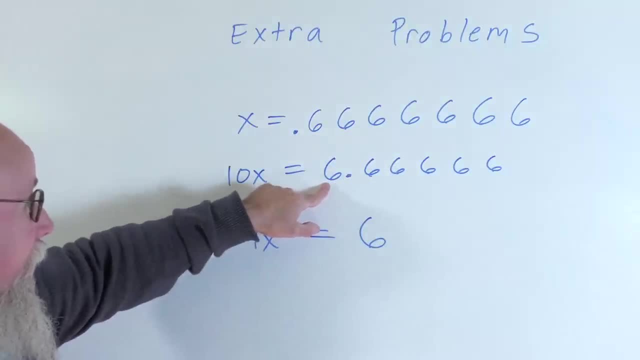 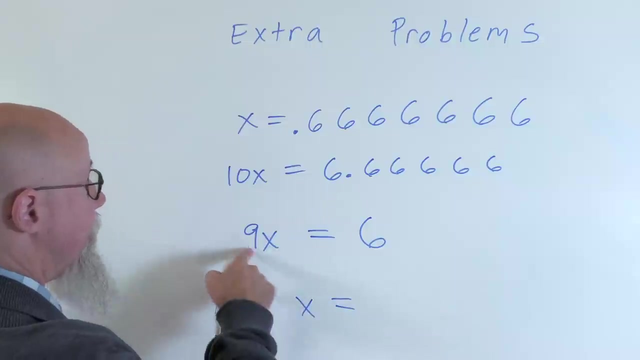 so multiplying it by 10 moves it over. now i have six point something and when i subtract 10x minus 1x is 9x, then that all cancels. and if i have 9x, how do i get to x? divide both sides by 9 so we get. 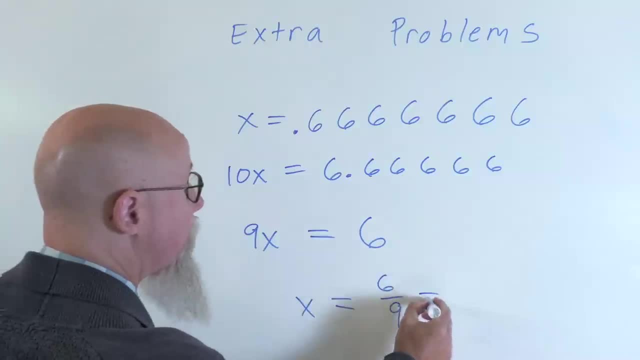 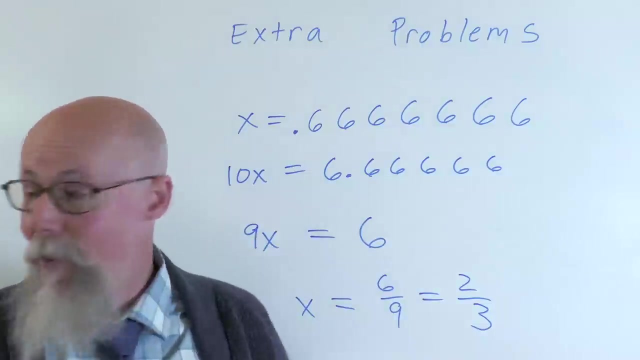 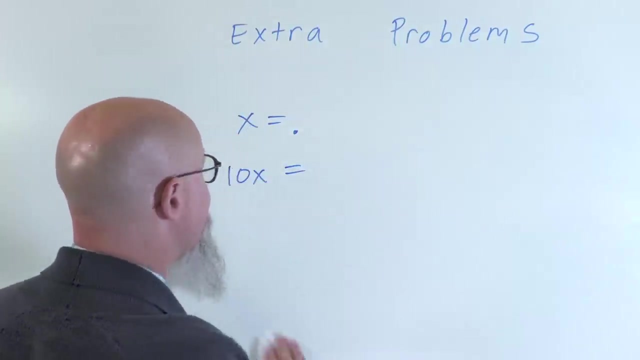 6 over 9.. which we know. then mathematically we can reduce: divided by three is two, divided by three is three, and actually this works. any single digit that repeats is a factor of nine. so if i have, if i have anything else, and actually i might use the same same formula, but if i have anything else, 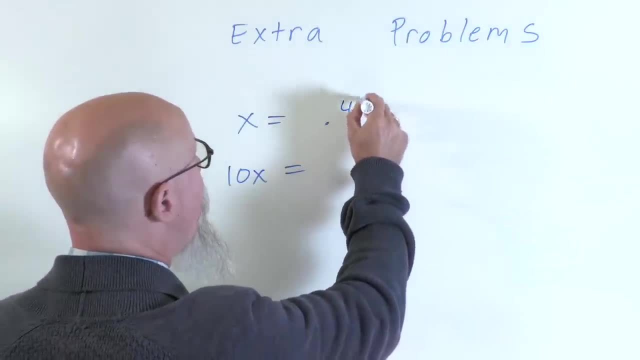 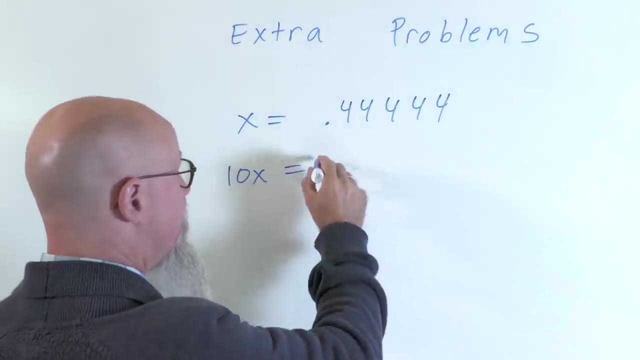 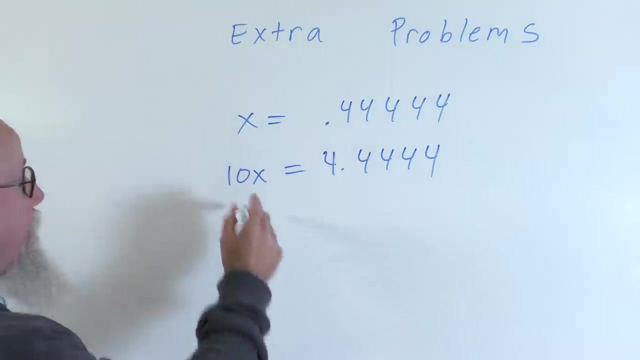 like if i have um point 4, and it's a 4 that keeps repeating, So then 10 times that would be 4 point, and as many 4's as you want. So then, when we subtract 10x minus x is 9x, and then when I subtract this, everything, 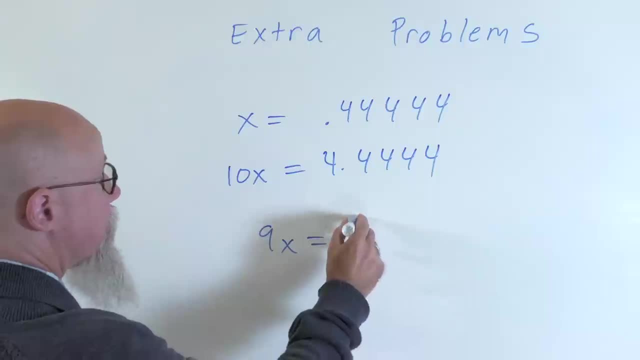 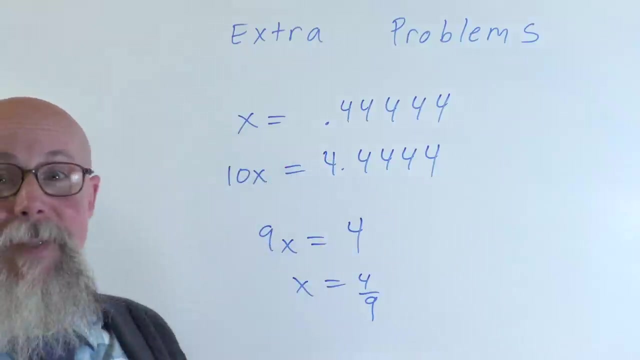 after the decimal subtracts, and so your answer is 4.. And divide by 9, x equals 4 over 9.. Now, so this works for any number 1 through 9, but this is kind of interesting then. 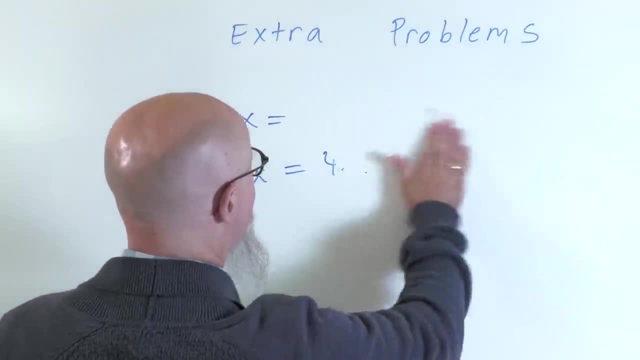 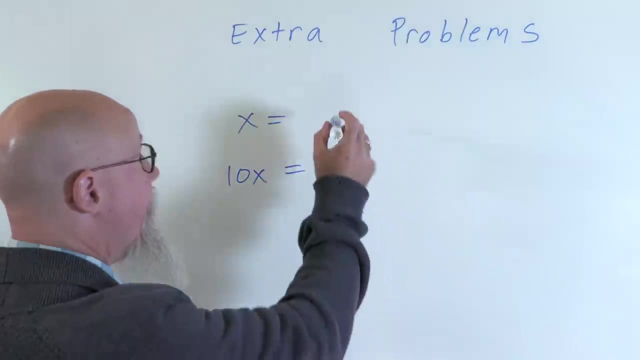 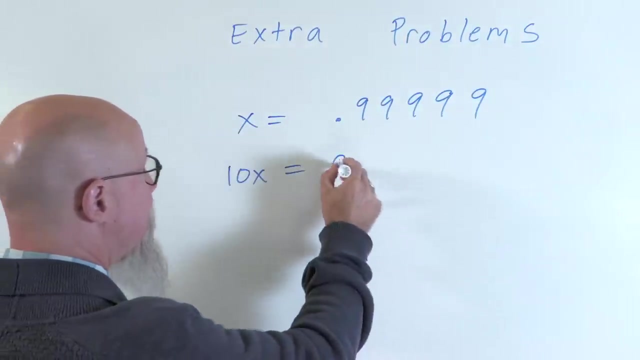 What if you get a 0.9 repeating? Because would that be then 9 over 9?? Yes, maybe. So if I have 0.9 repeating, and so then 10 times, that would be 9 point, And as many 9's as you want, we'll do the same thing. 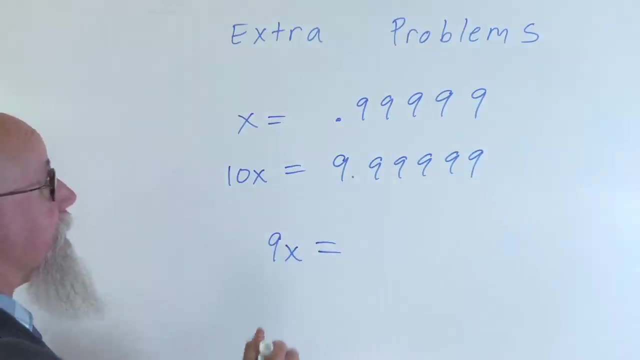 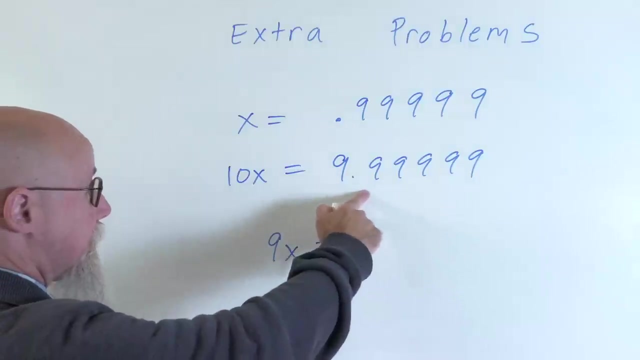 So 9x equals. so you see, if this is 0.9, repeating this still follows 10 times that, and then when we subtract it, all lines up, it becomes 9, x equals 9 over 9,, which is 1.. 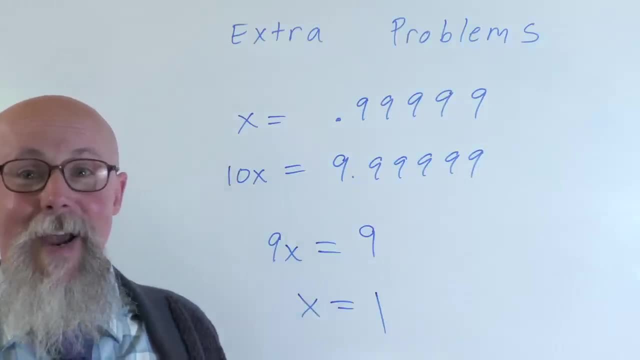 So you see some algebra acrobatics. How do I show that 0.999 repeating equals 1.. And these are kind of the things that we want to bring in, Some of the other things that we can do. you know, this works out nicely, just seeing it. 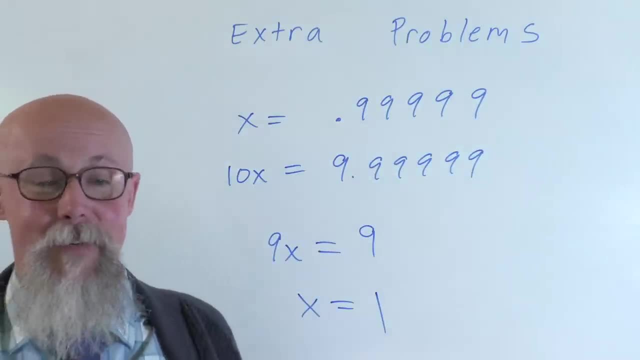 on the board. but later on, as we do different things to convert decimals to fractions, you can see that it'll work in the code too. But yeah, some math acrobatics. This is kind of what we want to be able to do. 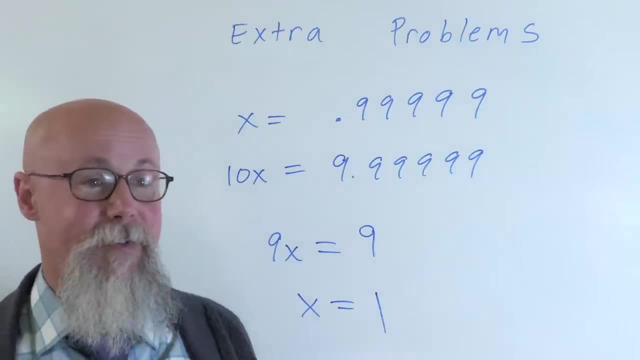 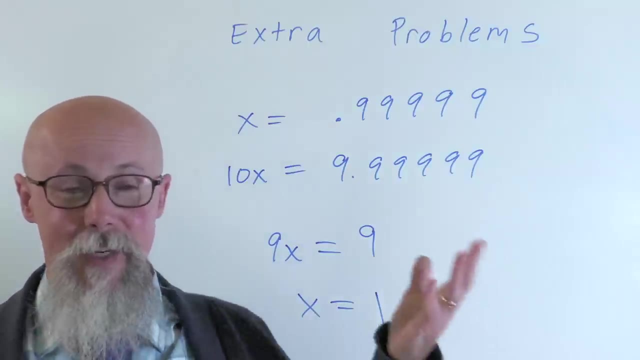 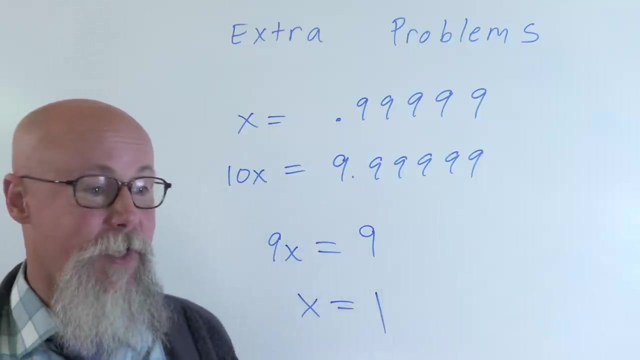 We want to also sometimes use the code to show different ways to get to solutions, And when we see it get to a solution In different ways, it kind of like reproves: hey, this works, this is the true solution. So these are some of the things that we can do with proportions, and you know some of. 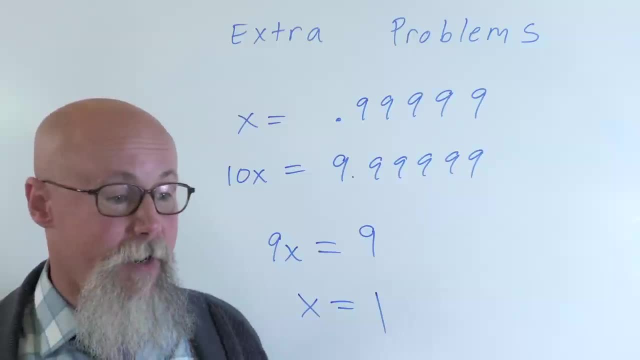 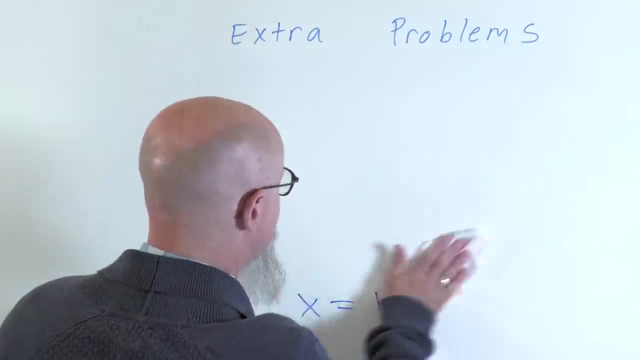 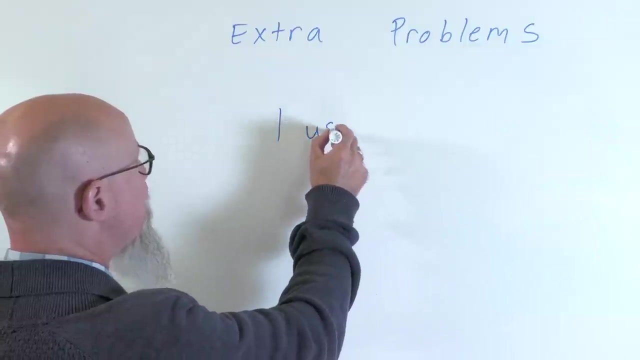 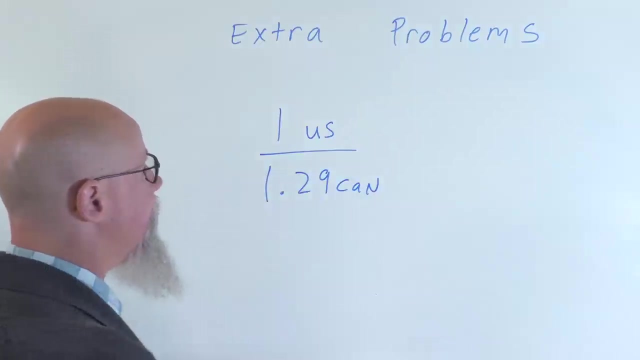 the other things we'll do. you know we could look at like converting money, like so, if I have, you know, let's say You know one US dollar is right now. I just looked this up, it's 1.29 Canadian dollars. 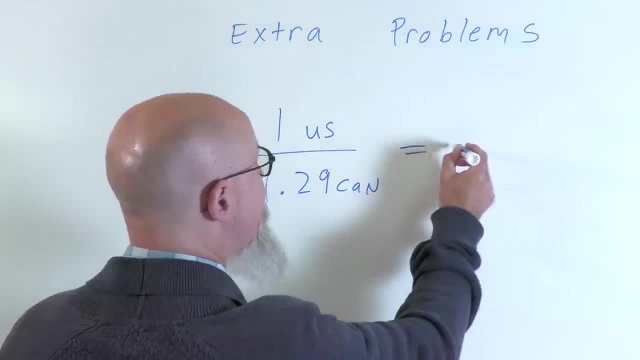 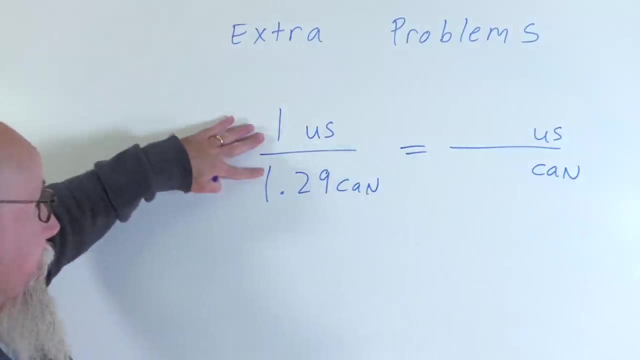 So if I want to convert, then I can set up my ratio and proportion. as long as you know, I know one of these, so I know the ratio And then, as long as I know one of these, I can figure out the other. 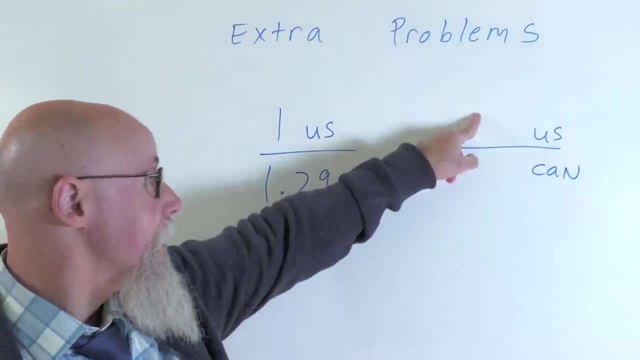 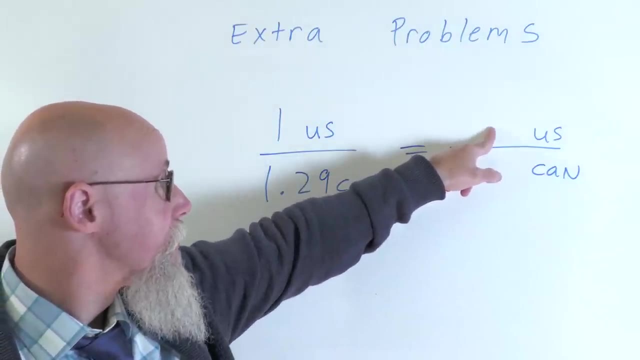 And in the code You remember, Just add it. whichever one I want to figure out, I put a zero there because either way, zero over anything is zero, So that would not apply here. You know the zero in the numerator. the answer is zero. 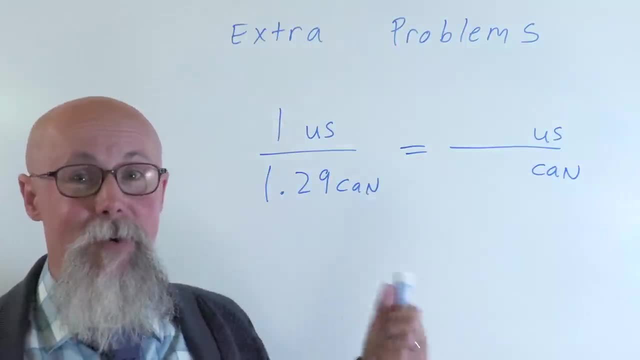 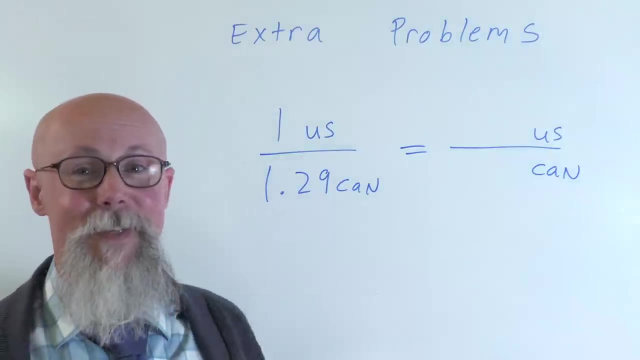 And zero in the denominator would be undefined. You know you could look up different images of divide by zero online. you know things like going into the abyss and all kinds of fun things like that. But yeah, we don't want to divide by zero. 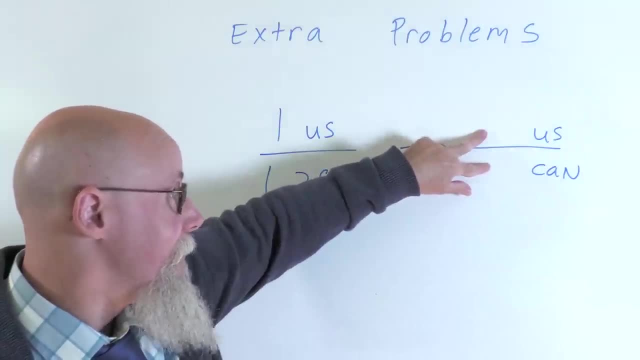 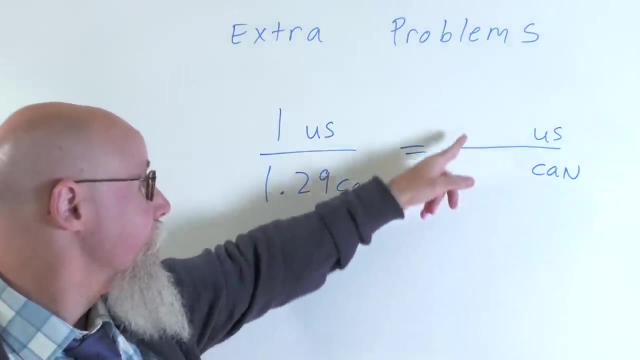 So if I know one of these and neither of these would be zero, that just really we would never arrive at that situation. So you know, we saw that. that's why we would put a zero in for the one we want to know. 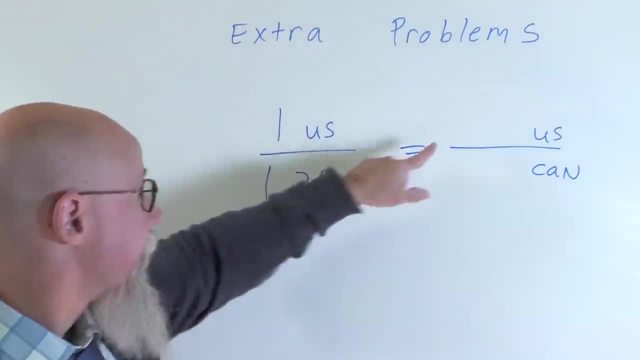 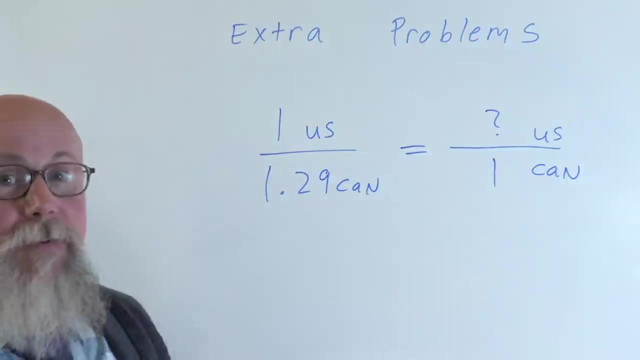 And there we go As long as we have it set up, you know, then I can figure out. oh okay, well, in that case, you know how many? I'll put the question mark here, since we're not in the code you. 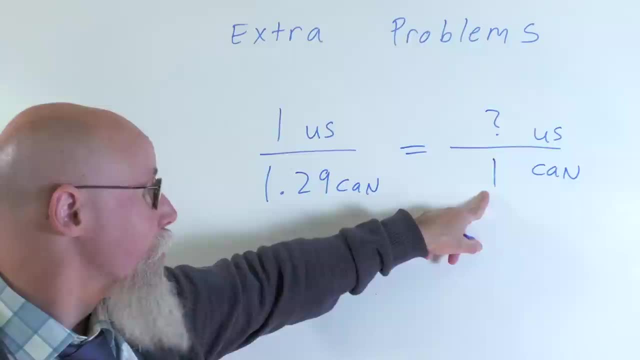 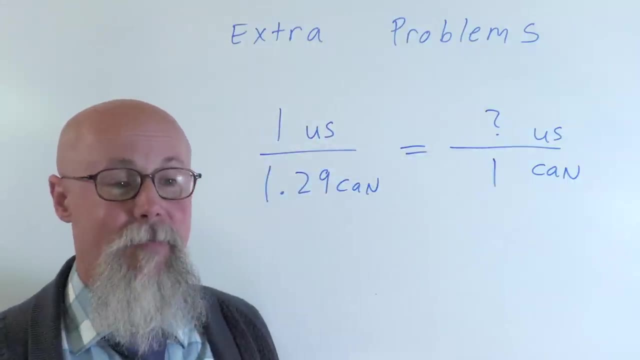 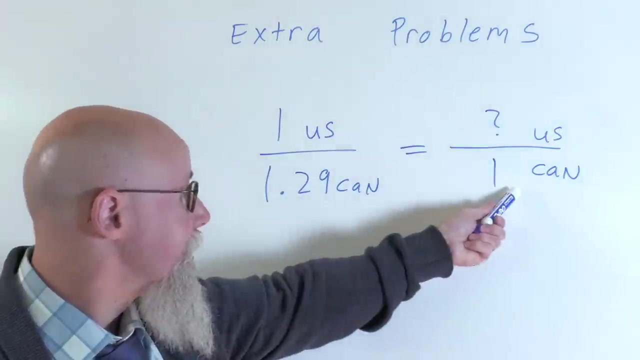 know, Okay, What's 1.29 Canadian, Then what's one Canadian dollar worth? And then you see, cross, multiply, divide by 1.29 and you'll get that exchange rate. So that's how we can change it from unit to this one. one US to how many Canadian? 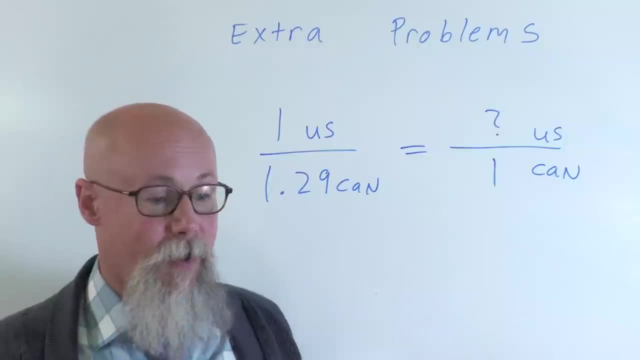 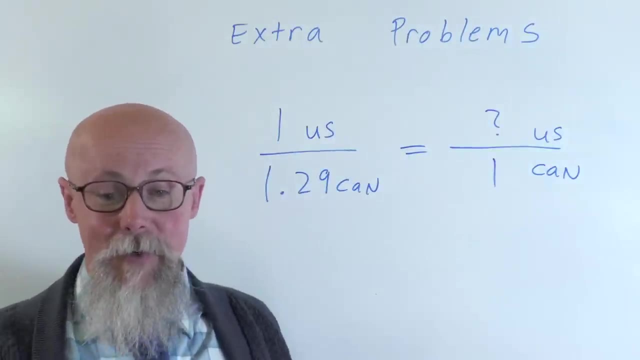 We can change it to one Canadian, to how many US you know? because very often you find exchange rates and they'll give you it in one direction and maybe you want to find it in the other direction. So these are some things you can use this for. 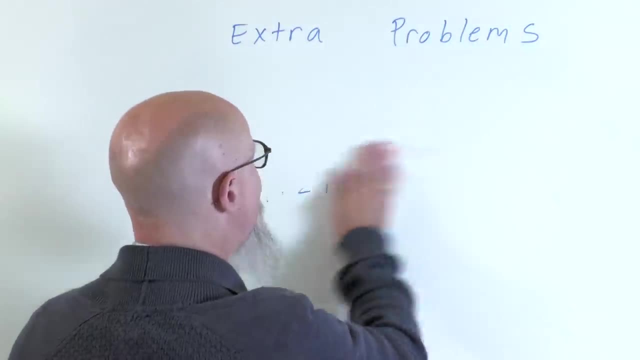 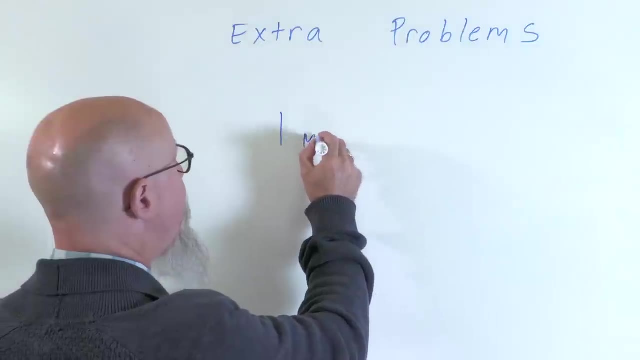 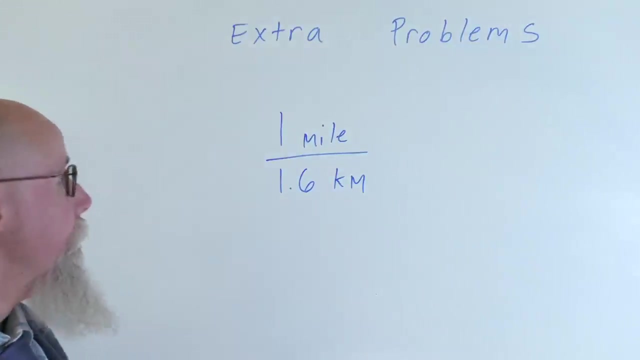 We can also do things. We can do things like miles to kilometers or or whatever you know other unit conversion you want. But you know, if you have one mile is 1.6 kilometers, um, it's not exactly 1.6, you. 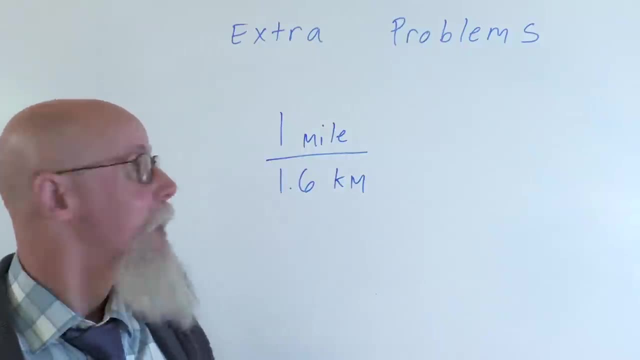 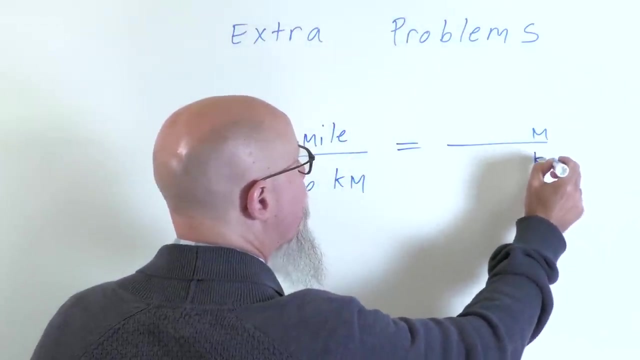 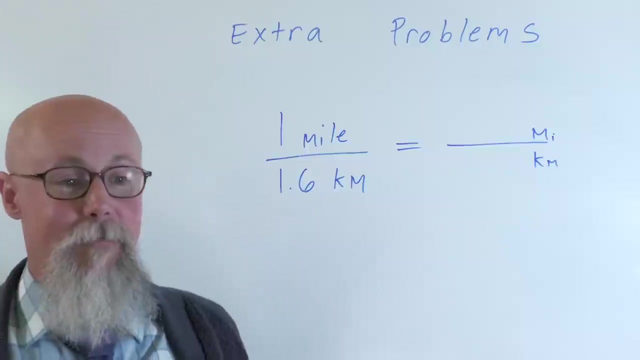 know there's, like you know, another nine meters or something, but okay, And then there we go. If I want to convert, then as long as I have miles and I have kilometers, Then it'll work out. And we looked at how to put that in the code. 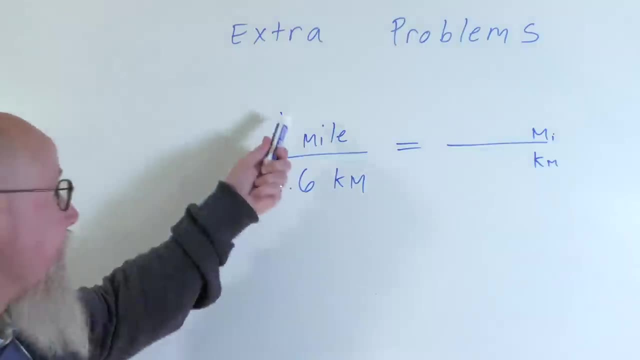 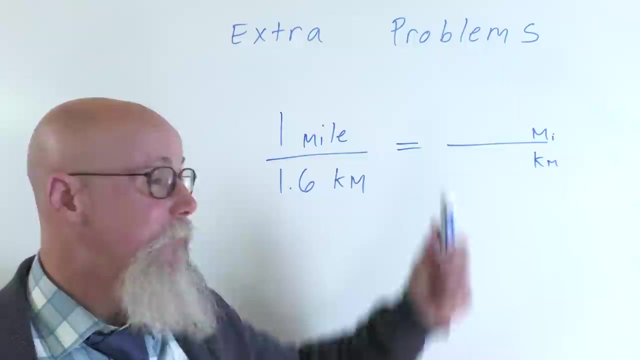 So, now that you have these tools, you can convert anything. As long as you have that ratio of one aspect of it, then you can, you know, plug in one of these two numbers and figure out the other. So you know here, you know some, some of the good things, and these are some of the 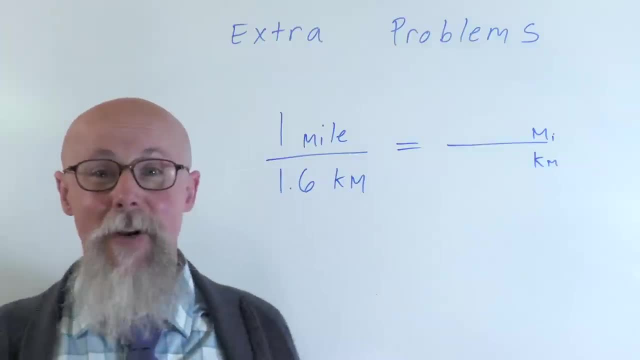 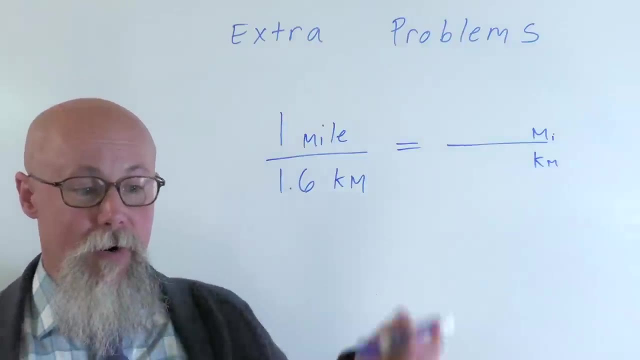 things we wanted to do in the extra practice section. You'll see this come up in every unit Um that you know we're going to get to the core um, core skills and those units are going to build your ongoing uh Colab notebook. 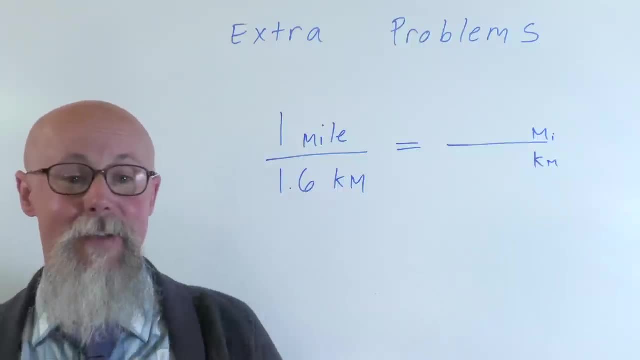 So you have some resources and then we'll have an extra practice, um, extra practice, extra problem section, where we then use some of the things that you've created and let's apply this and let's solve a bunch of extra problems. So there we go. 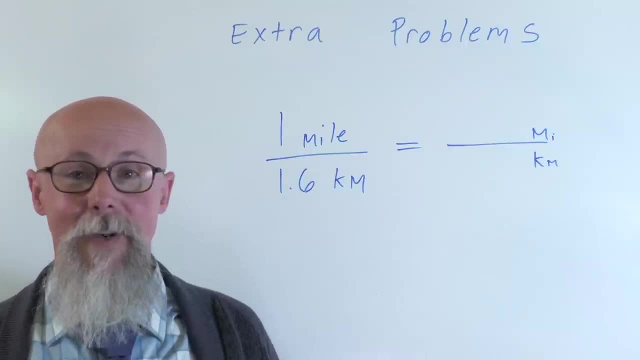 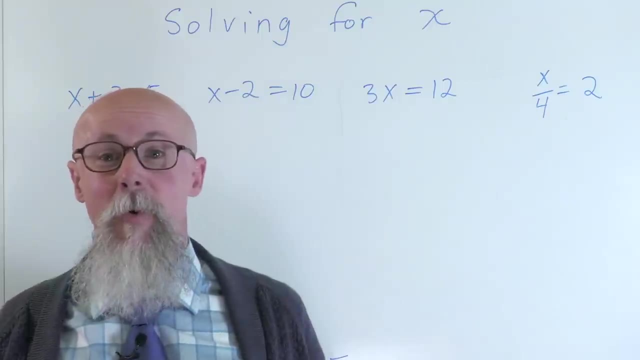 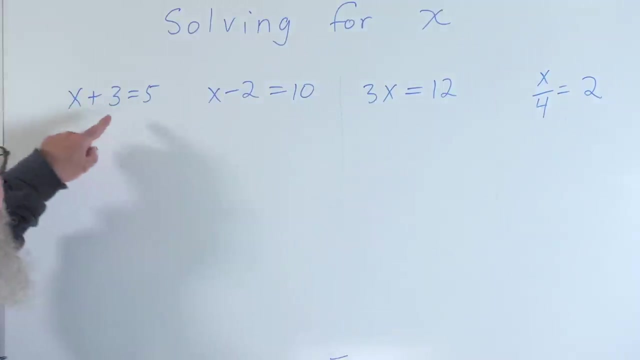 Um and we will, uh, we'll go on, We'll go on to the next unit. Here we're going to look at four different ways to solve for the unknown number, And in algebra we often call this X, just because X works nicely. 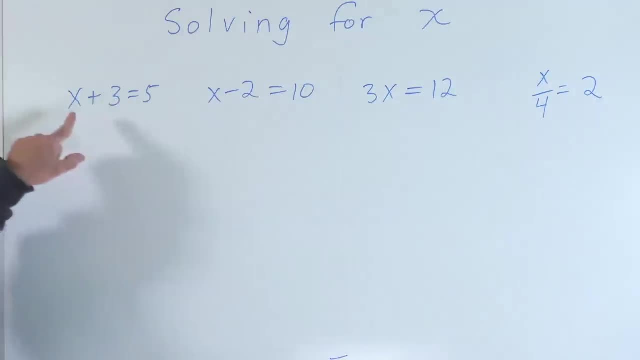 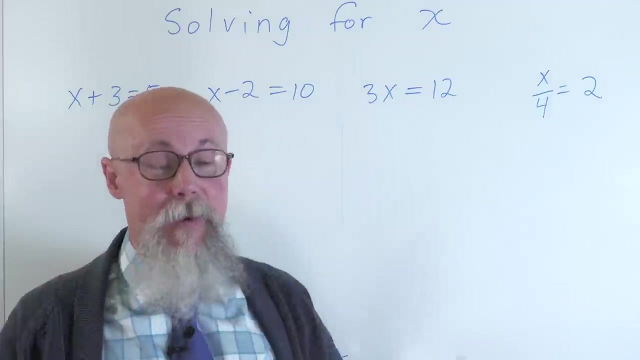 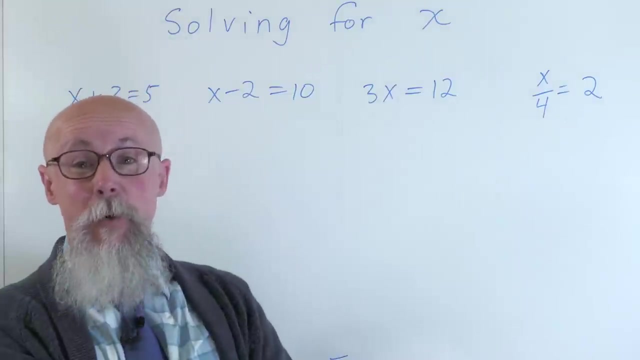 X marks the spot. So if I have, I had to put four different situations here: add, subtract, multiply, divide. So I put simple numbers because you might be able to do this in your head to see the answer. The algebra explanation is: you want to see what you're doing and do the opposite. 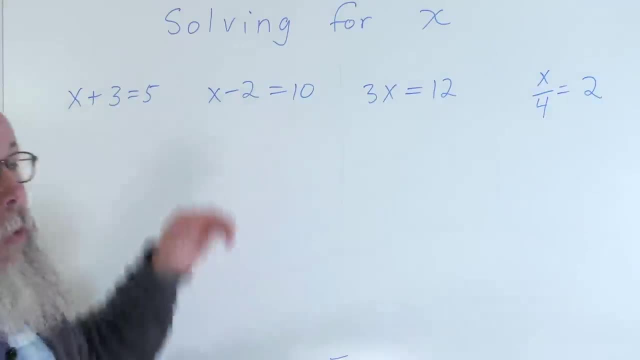 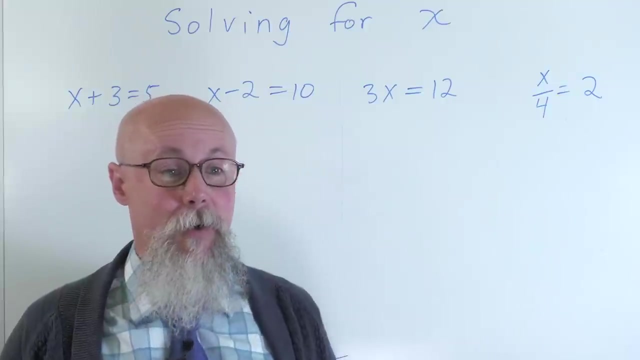 So then, if these two sides are equal, both sides of the equal sign, if you do the same thing to both sides, then they stay equal. So that works. What am I doing? I want to do the opposite, to cancel things out. 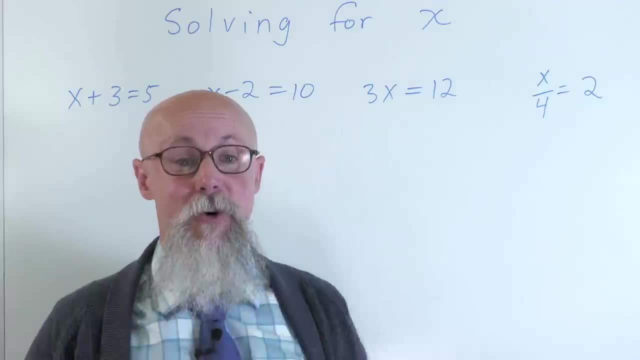 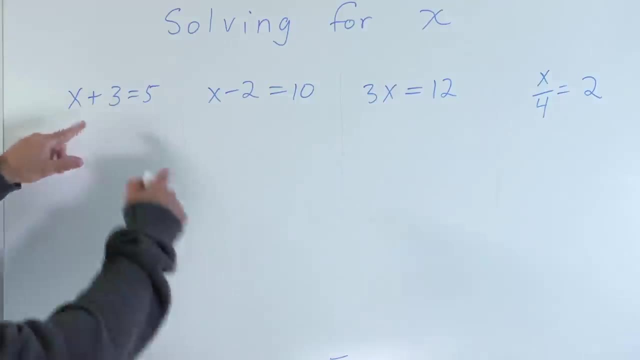 Then the next thing is do the same thing to both sides of the equal sign. I'm going to show this with the four different algebra operations here. So I have X plus three equals five. So in each time the goal is that I get X equals something. 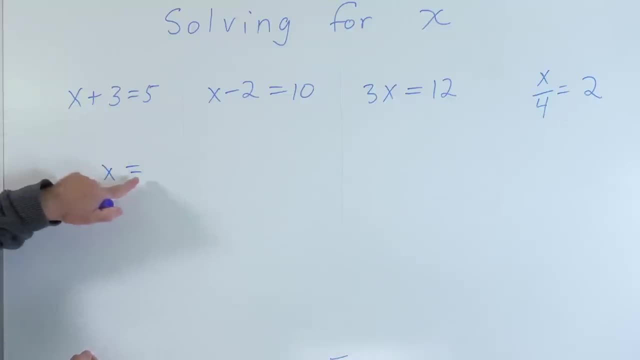 So I would like that X by itself on that side, on the left side of the equal sign. So what am I doing? I'm adding three, So I'm going to do the opposite: subtract three, and then I'm going to do the same thing. 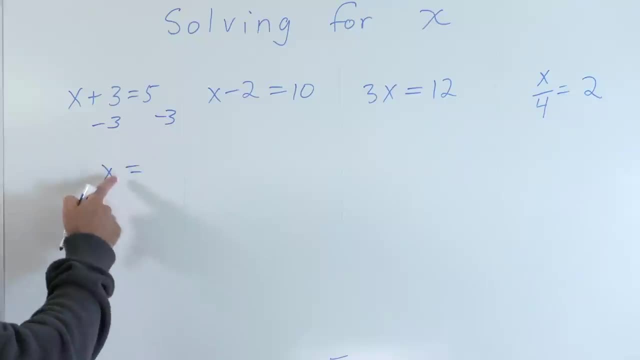 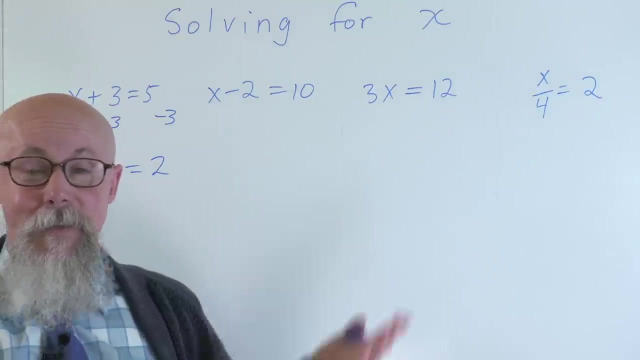 to the other side, And three minus three is zero. I don't have to write plus zero, Five minus three is two. Solved X equals five, X equals two. So it's like Sherlock Holmes eliminating possibilities, and then we get to the answer. 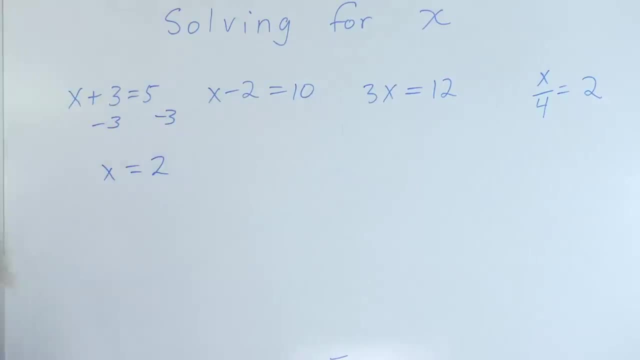 So the next one: if I'm subtracting, I'm going to do the opposite. So again, my goal is: X equals something, So X minus two. if I add two, that cancels. That's why I add two. And then I do the same thing to the other side. 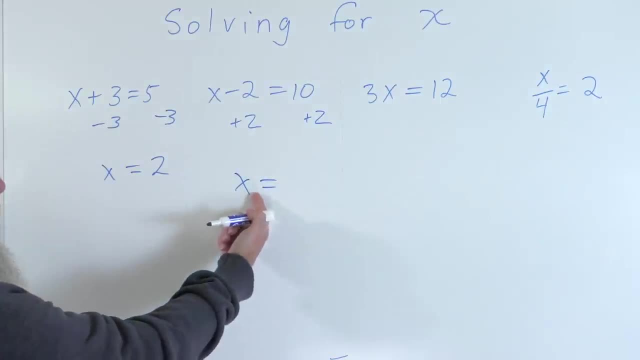 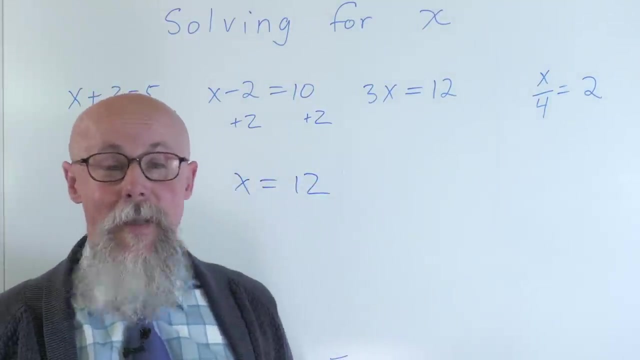 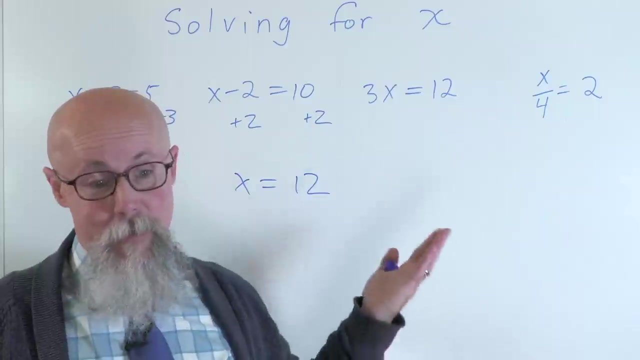 So negative two plus two is zero. Don't have to write plus zero. And then 10 plus two is 12.. There we go, Solved. We go to multiplying. Very similar. Also, notice in writing math: most textbooks you won't see the fact that you won't see. 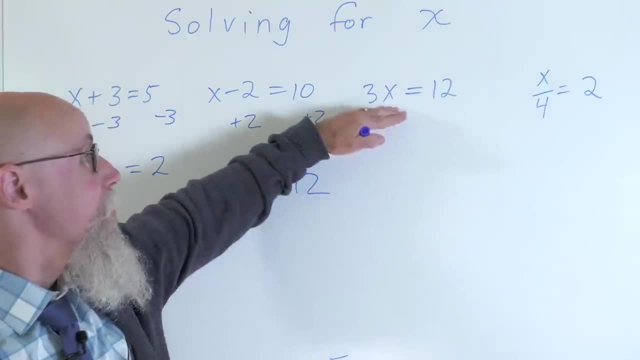 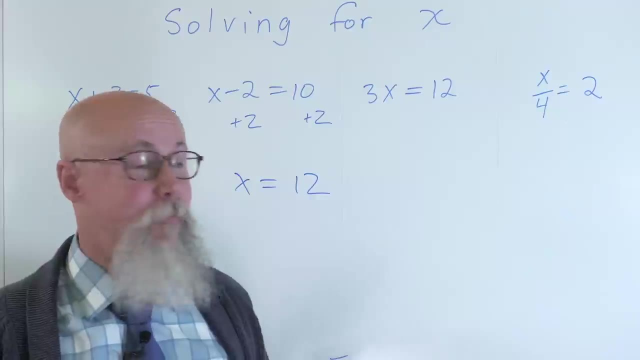 a multiplication symbol at some point. Just the fact that they're next to each other means that I'm multiplying. Now we have to remember this. in Python syntax you have to put that multiplication symbol. But here three X means three times X. 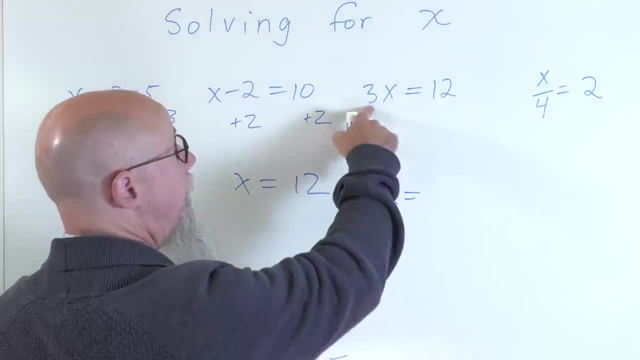 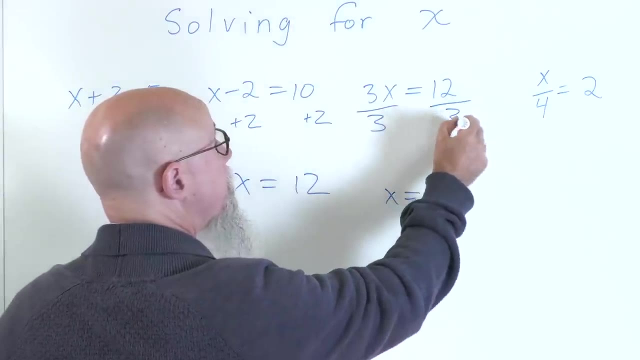 So to get X by itself, I'm multiplying, so I have to want to divide And notice. I'm going to write that like a fraction divided by three and then divided by three here. Now here's something else about the notation. 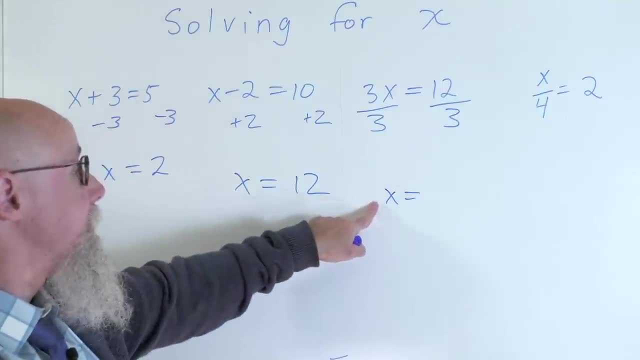 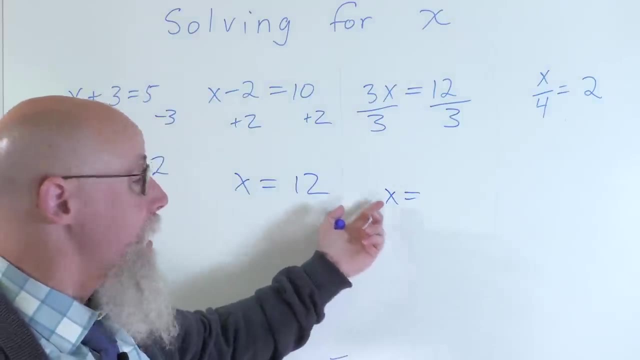 Three divided by three is one, but I don't have to put one X. You could, but you don't have to And most places you won't see it. You know one X. Any other number there I'd have to write the number, but one we often don't write. 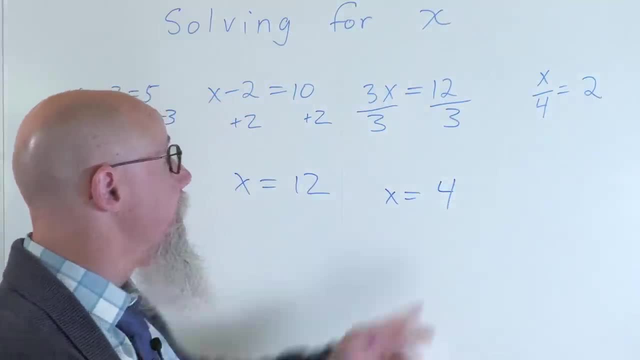 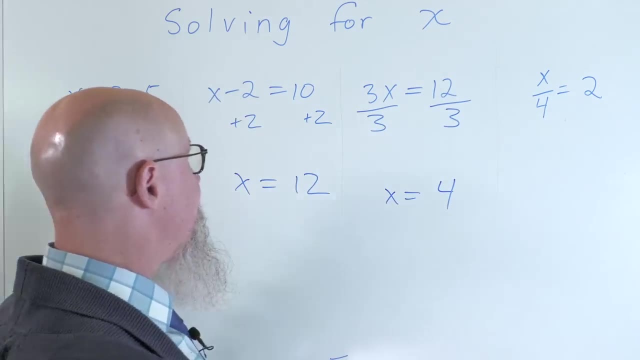 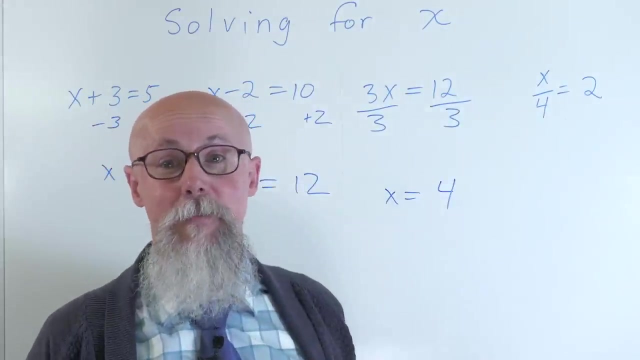 that. So 12 divided by three is four, And we go here: X divided by four. somehow, whenever I teach this, everybody's like: get it, get it, get it confused. It's the same thing I'm dividing, so I'm going to do the opposite, which is multiply. 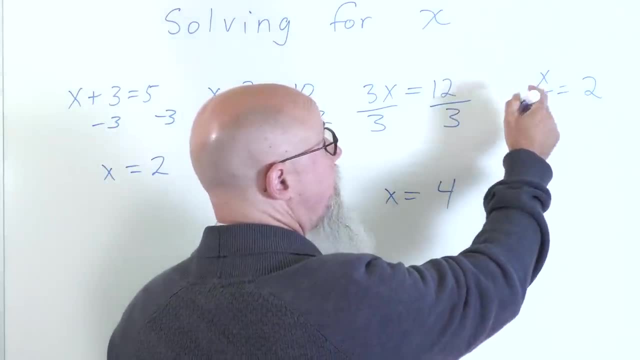 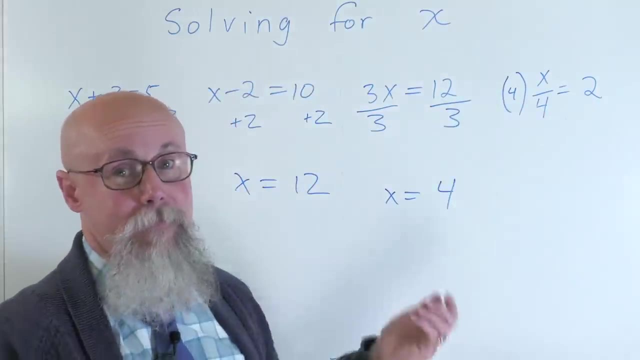 Now, in this case I might write it- you know how can I write: multiplied by four. I might even just put it in parentheses, just saying it's next to that. so that means I'm multiplying. That's one way to put it. 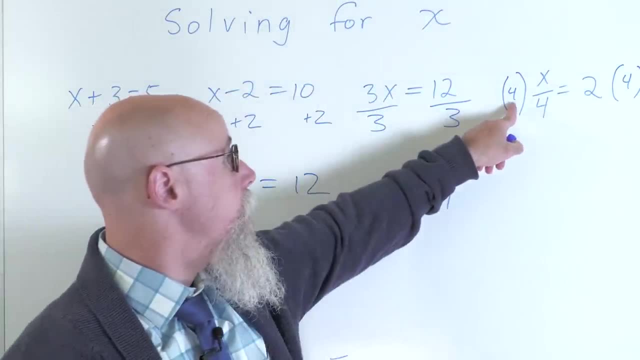 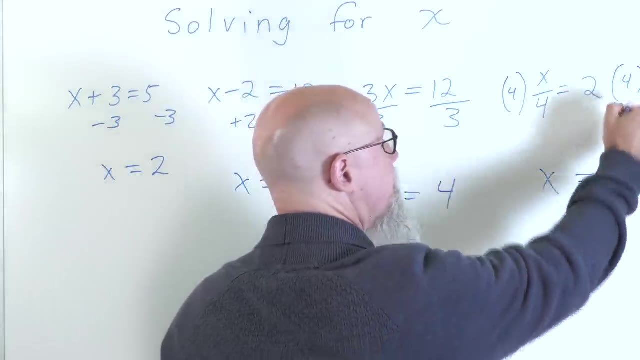 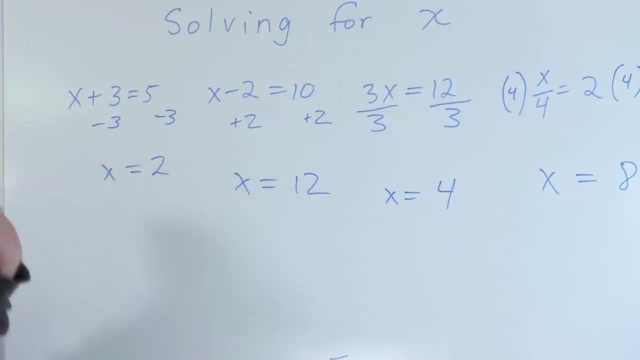 And so here I'll put it in parentheses: So divided by four times four cancels out, so it's one, and then that's one X, And then here two times four is eight. So with some simple numbers that you know, we see these methods here: add subtract. 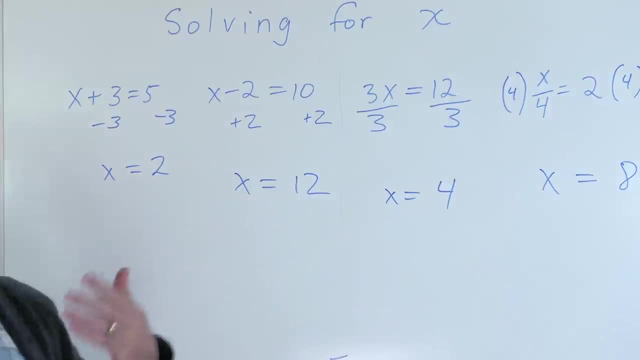 multiply and divide And the key is: no matter what the numbers, no matter what else you encounter, like how complicated the numbers are, It's the same method. So we recognize this method. then whatever number comes up, then we can figure this out. 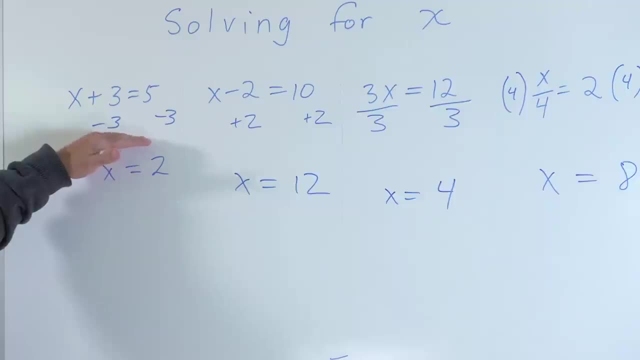 Because this I can do in my head. but supposing I have, instead of X plus three, supposing I have, you know X plus you know 7.2, you know equals 11.1, or something like that. 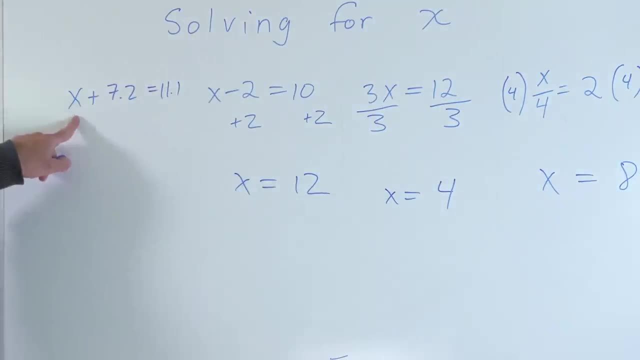 So, supposing, if, I, Supposing, I have something like this, how could I solve it? Oh, I have an algebra method to it. What am I doing? I'm subtracting, in this case 7.2, from both sides. 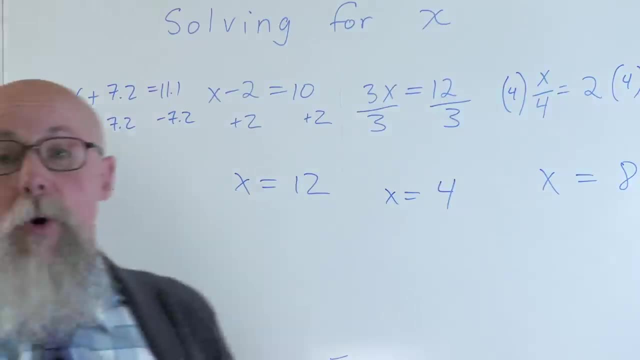 And so then I get X equals. and even if it was something more complicated, I know what I'm doing on the calculator. I'm subtracting 11.1 minus 7.2, and then I know what I'm doing on the calculator. 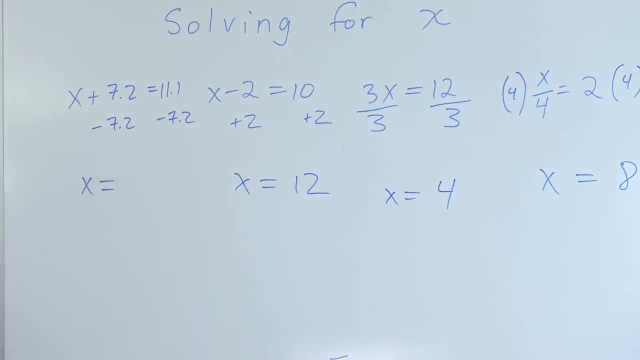 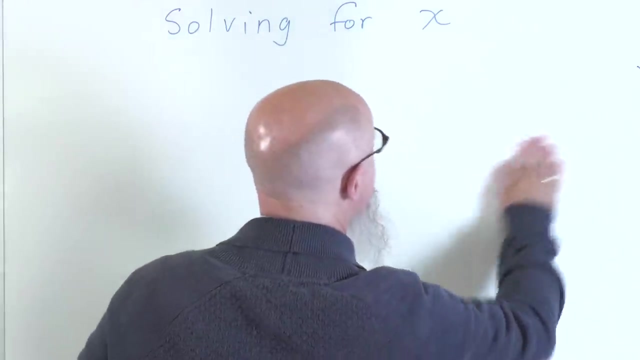 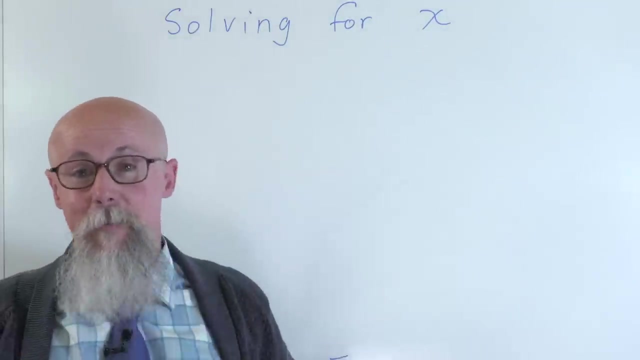 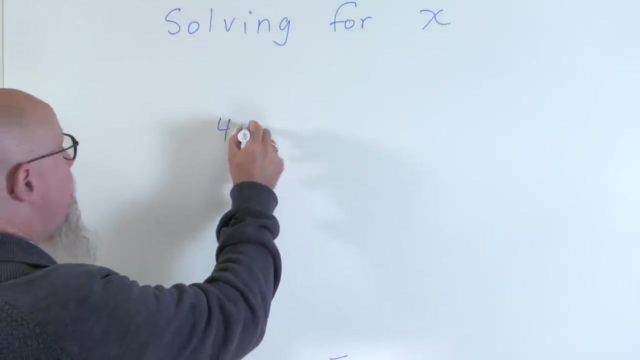 There we go, So we can also use this anytime. I have, you know, a two-step equation And in the two-step equations it's more, like you know, order of operations in reverse, because the addition's the easiest. So if I have something like you know, 4X plus 6 equals 22.. 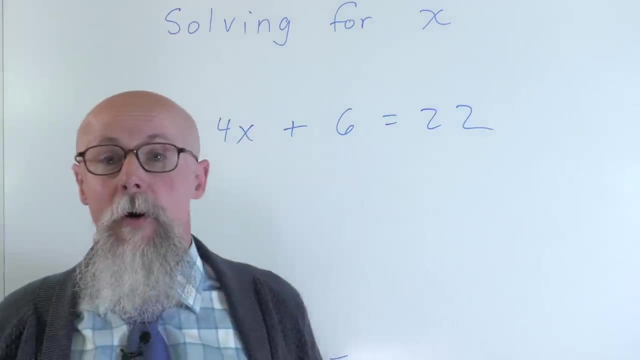 So I'm subtracting, and even if it were something more complicated, I know what I'm doing on the calculator. So two steps I'm still going to combine those same four steps we were talking about. I'm just going to do one, then the other. 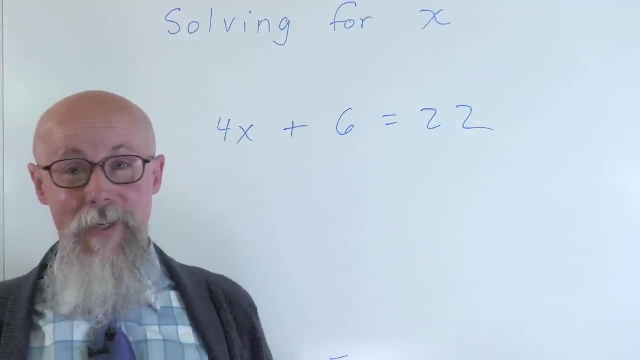 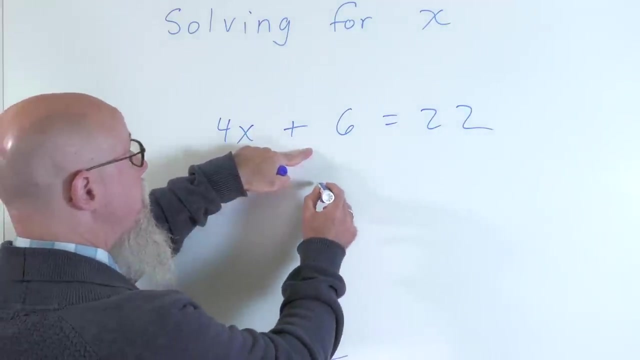 And I'll look at the addition like I said, like order of operations in reverse. the addition or subtraction is going to be the easiest to do first, If I then subtract six from both sides, so if I have minus six, minus six, so then I. 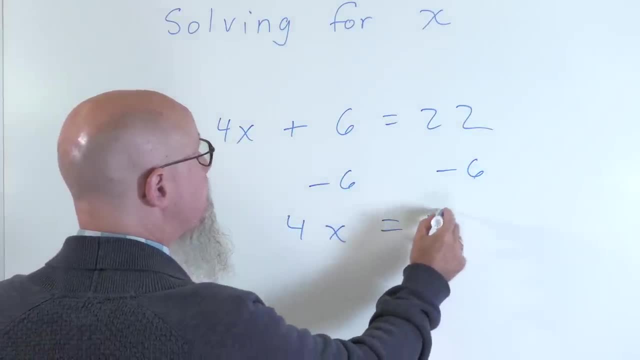 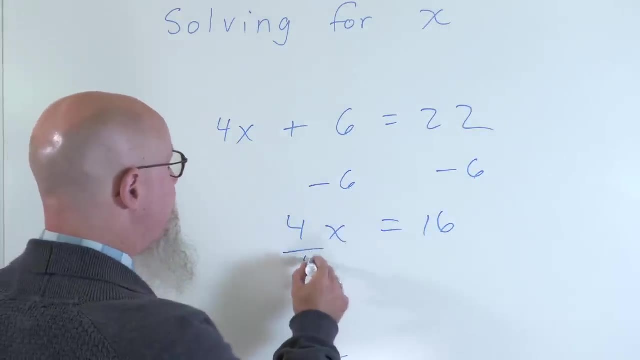 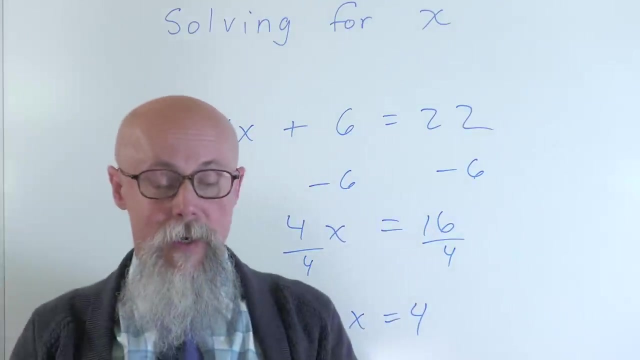 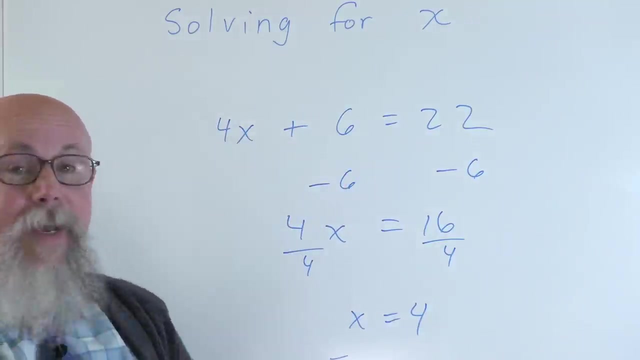 have four, x equals 16.. And now I get to my second step: divide by four, divide by four, divide by four, then I get x equals four. So we have our two step equation. And in all of this, some of these are, you know you're going to get quick enough at. 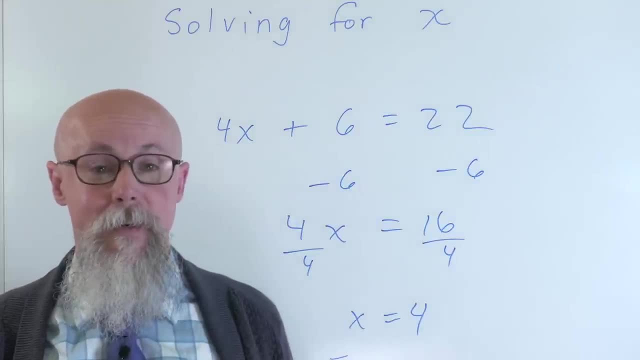 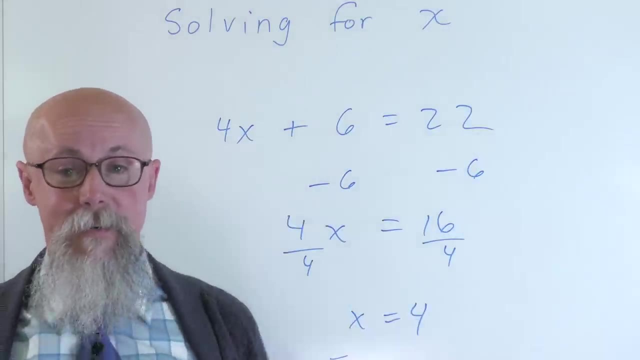 this that it's not even worth trying to write code or anything to solve this. But some of these, as they get more difficult, then it will, you know, and there's other factoring and you know more elaborate problems, then it'd be worth it to write code because 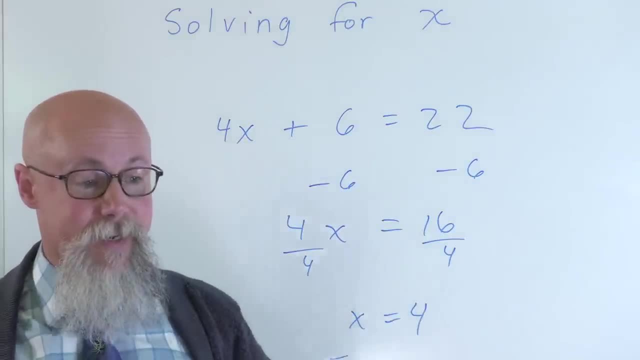 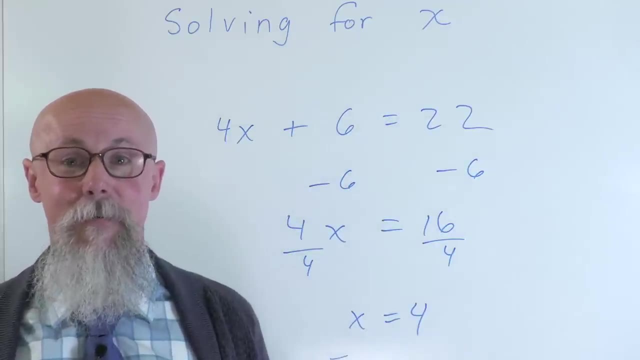 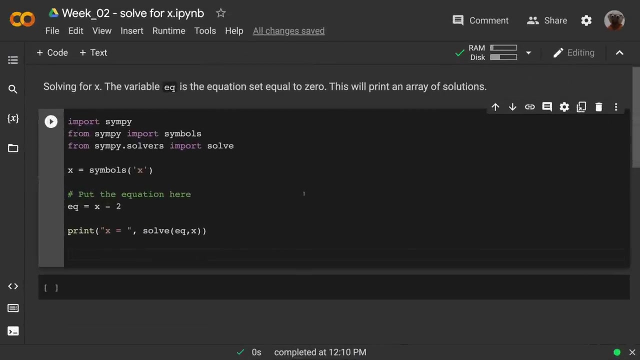 we'll show. I'll show you now how we can just put this in in Python. write out the equation and it'll output the answer. So let's take a look at the code. So it's a lot easier to solve for x in Python because we can just 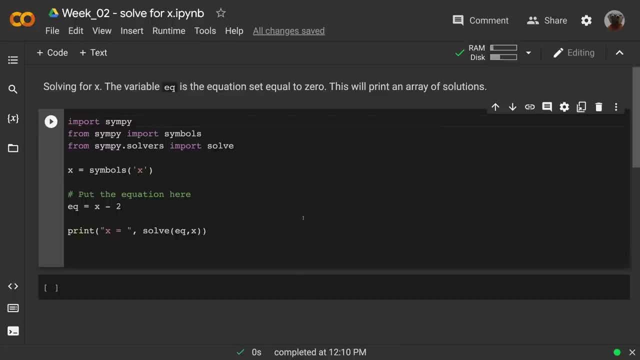 import the SymPy library here And that's the symbolic math library. you don't have to install anything, you can just import it. Google Colab works nicely behind the scenes like that, And then from SymPy we're going to import symbols. 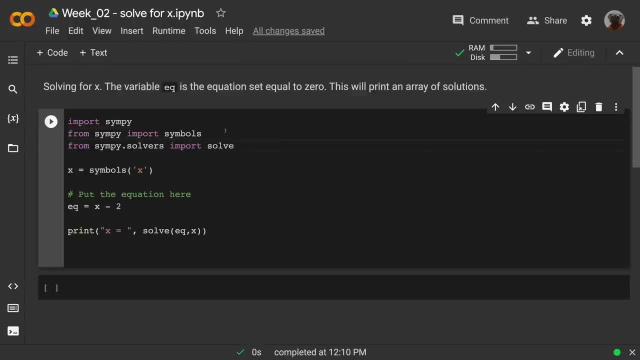 And from SymPysolvers. we're going to import solve, So we can import symbols to use x as a math symbol and solve for that, And solve is going to be the function we use. So we see here, then I'll define: x equals x. 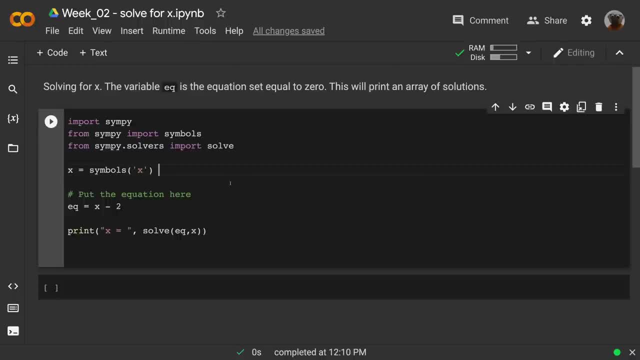 And that's defining that. x is the variable we're solving for. I just put this comment here. But then the next thing we have, I define this variable: EQ equals x minus two, And this is the function set equal to zero. So it's x minus two equals zero is what we're solving for. 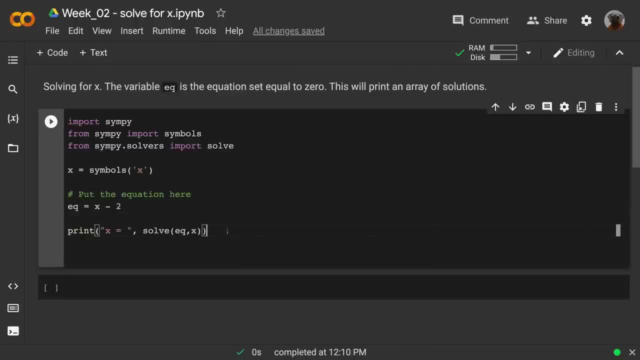 And then that's the equation. So then I just put it in a print statement: print x equals and Python syntax, Then we're done. Then print that exactly comma. and then our answer. And here's where we see: solve EQ, the equation and use x as the variable. 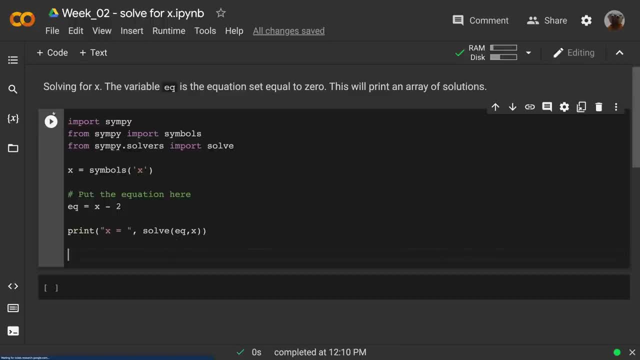 So we're going to solve that x minus two equals zero And you see it outputs x equals two. It will print an array of whatever your answer is. this just had one answer, But if I had something like x- x squared, I'm going to print that. 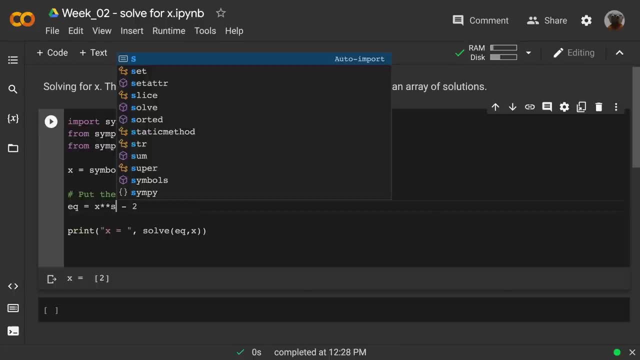 x squared, x squared minus two. Now that'll give me a square root answer. Kind of interesting how that'll show up. you see the square root of two rather than try to make that a decimal. But if we make this something that works out nicely to an integer- and we've run that- 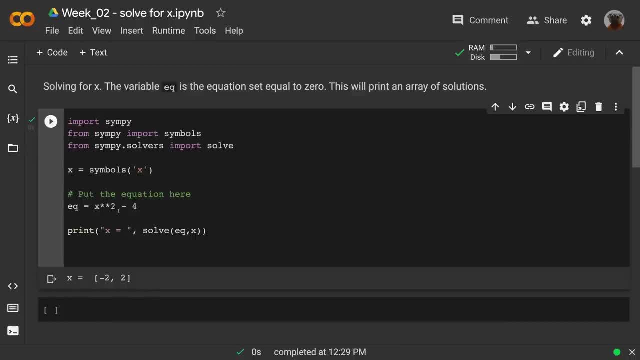 see, it'll give me an array of. you know my two answers: x squared minus four equals zero, is the equation. And negative two or positive two, either one works. And remember then, if I have something like two x, I can't just write two x, I have to. 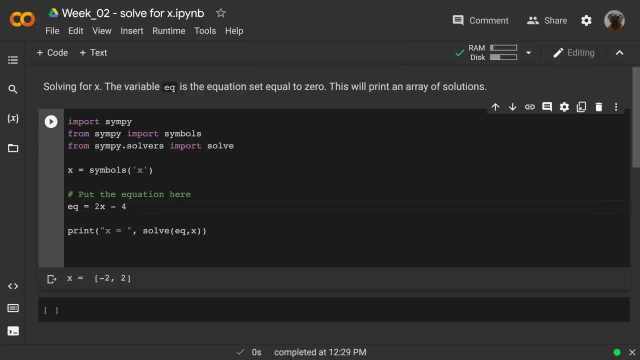 put: I have to put two times x, because that's Python syntax, two x minus four. And then if we run that, there we go. it'll solve that. There we go, Much easier. All of this stays the same. 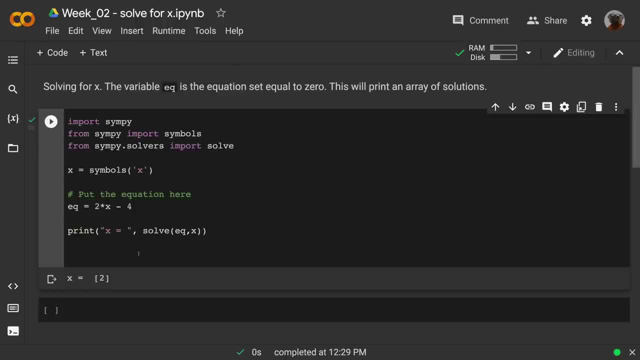 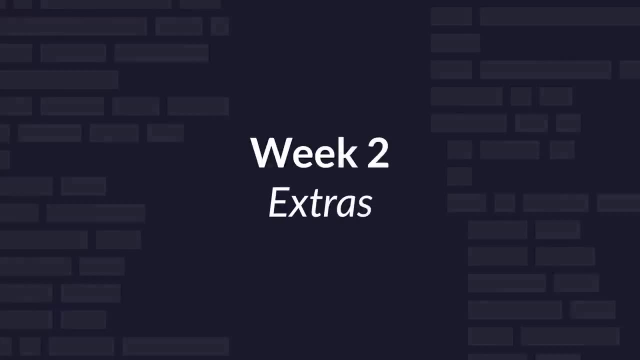 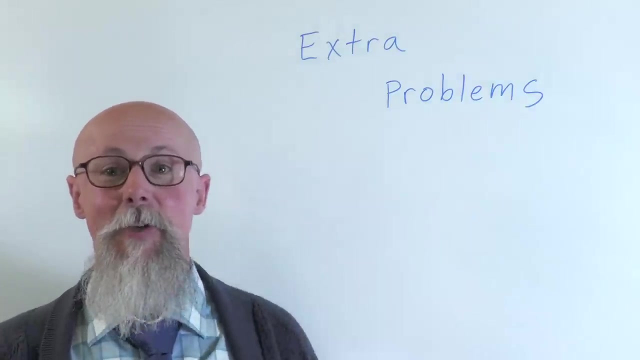 You just put your equation here and run it and you can solve anything, you know, just make sure it's set. it's that equation set equal to zero. Now that we've worked through the core skills in this unit, let's look through some extra. 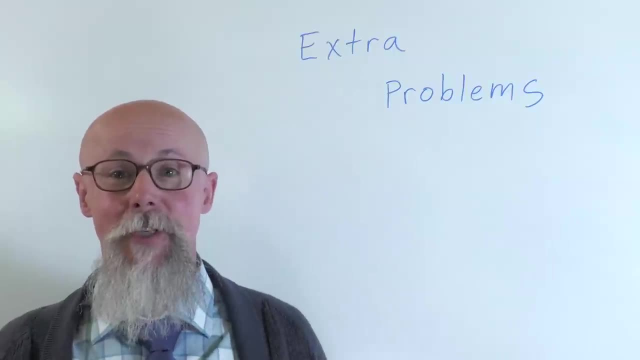 problems and I'm going to work through extra problems using the Colab notebook So you can see how you can apply these resources that you're building. Okay, So we're going to use the use these to solve problems that might come up in a textbook. 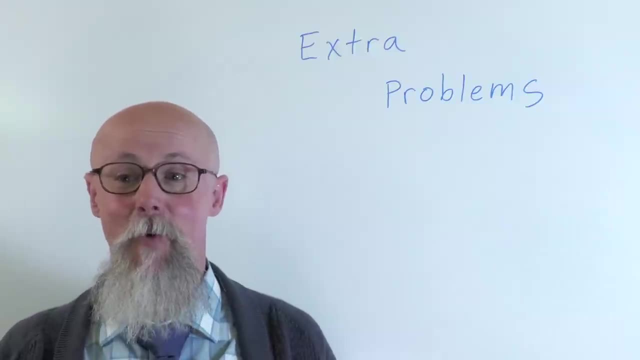 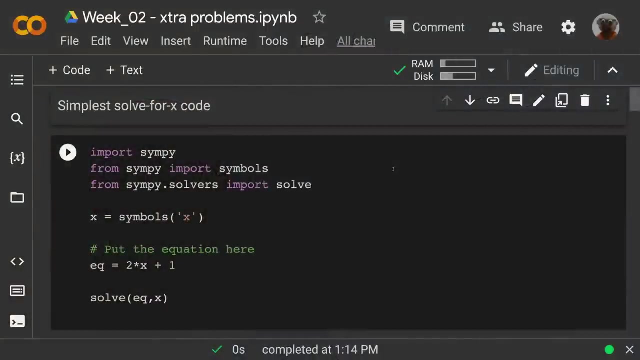 or in day-to-day life. So we're going to go through some more extra problems here, All right, So let's go a little bit deeper, looking at different ways we can solve for x here using Python code, And here is the code that we were talking about before. 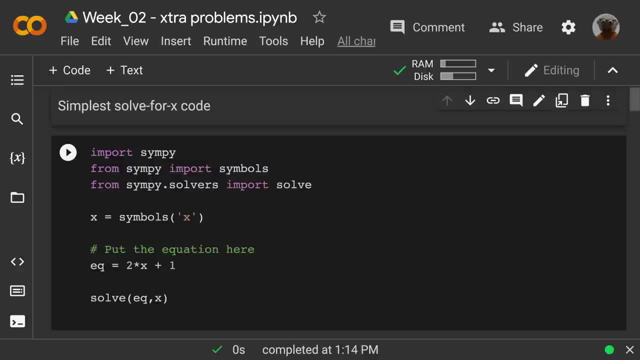 So we import SymPy so we can use our symbols, and then we're still from SymPy import symbols and SymPycom. Okay, So we're going to go to SymPysolvers And here I'm just going to define that symbol x, and this is the simplest thing. 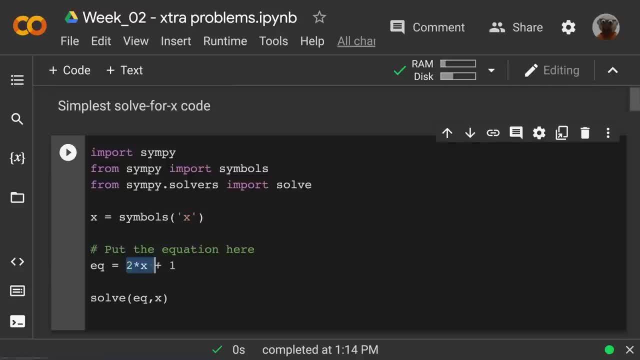 We can have all of this code and I can just put my equation right here- Here's my equation- And then I can solve that equation. and I'm solving for x. Notice, I don't even really need a print statement as long as this solve function is the last. 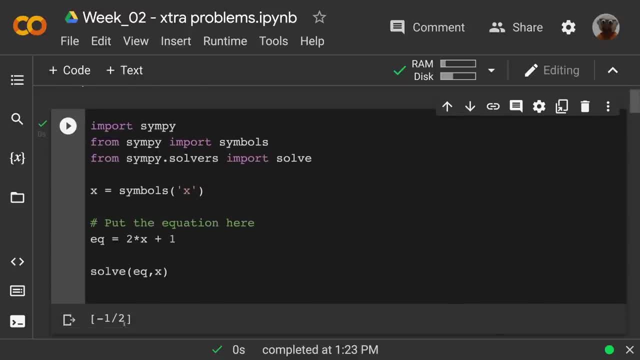 thing there And then when we run it, we see, Okay, It will give this negative one half And notice the brackets around it because it's a finite set. Nice, Solve, pretty easy. And if I have something that solves for even you know something more complex like two. 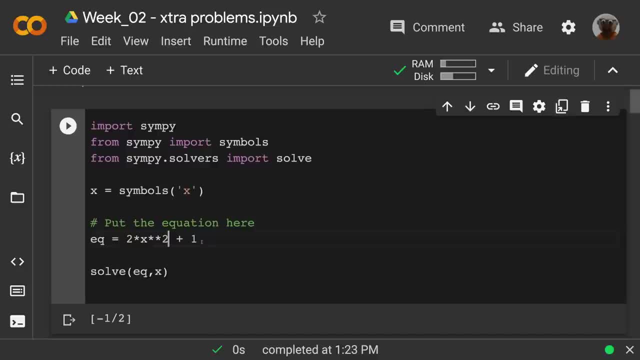 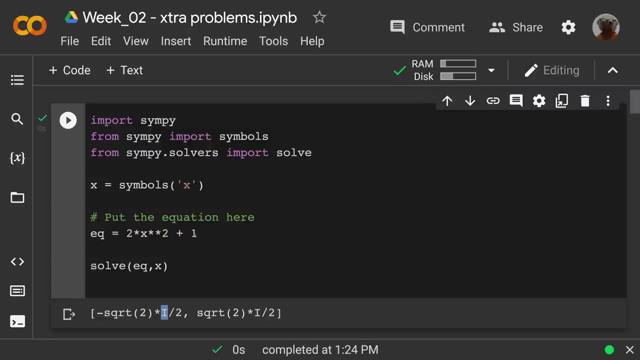 x squared plus one. Now this is setting this equal to zero. So two x squared plus one. Okay, And then this is where we actually won't have a real solution. We can actually take a look at that And you say the negative square root of I, and that is I, the imaginary number. 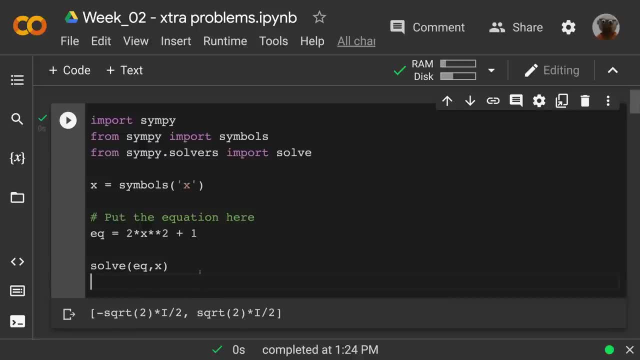 So it will give us this. There's other ways to Make that square root display in its better way, but we'll get to that later. and there we go. We see, You know, it gives us two solutions As this, And if I were to make it, you know minus one, or I can even make it minus, you know four. we'll have two real solutions there, but there's still going to be square root solutions. 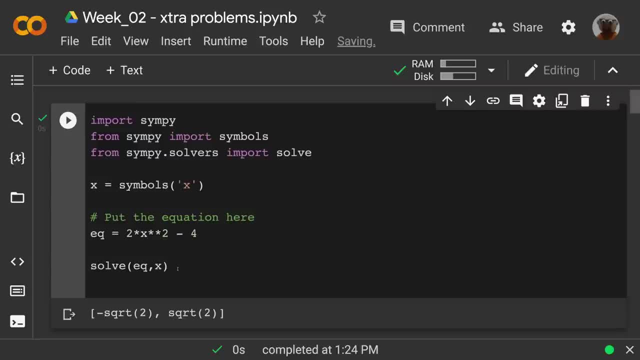 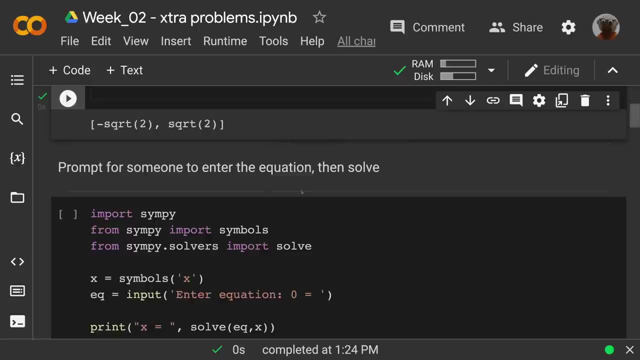 There we go Different ways that this will output, but you get this. You can put the equation in there and see the answer. It'll solve pretty much anything you can type in there. All right, But let's start making this a little bit fancier. What if we prompt for input? 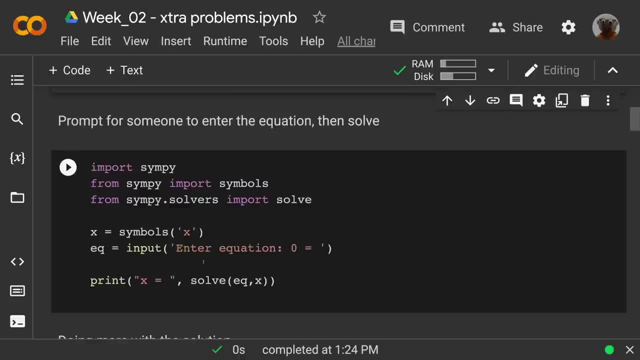 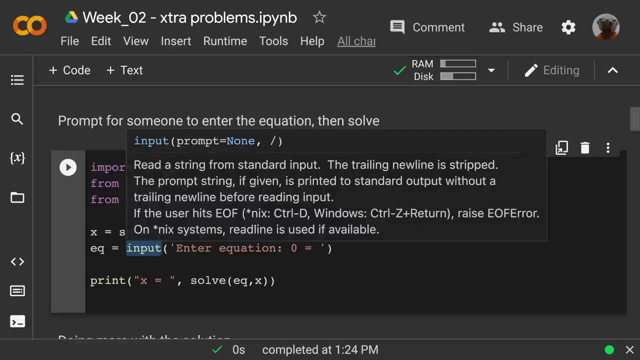 So let's say, I want this to be, you know somewhere else, and rather than somebody going in and finding that correct line and putting the code there, we can just prompt for the input here And notice the function is input and then it's going to display this: 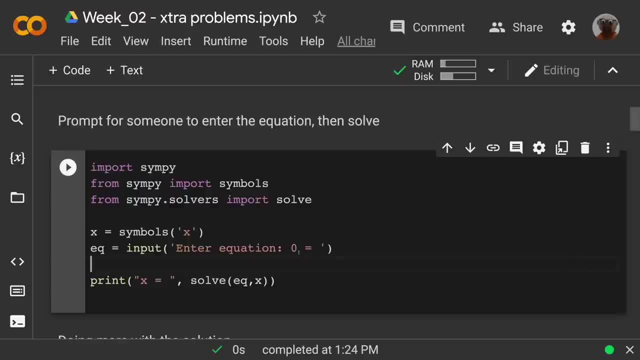 Enter equation and I even have it as zero equals. to remind the person that it must be equal to zero, You could add another print statement saying make sure X is the variable. you know if that's what you'd like- And this input does come in as a string, but the fact that we are using these symbols, it will be able to interpret that. 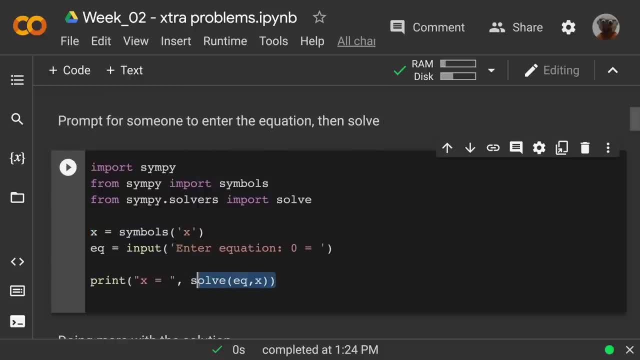 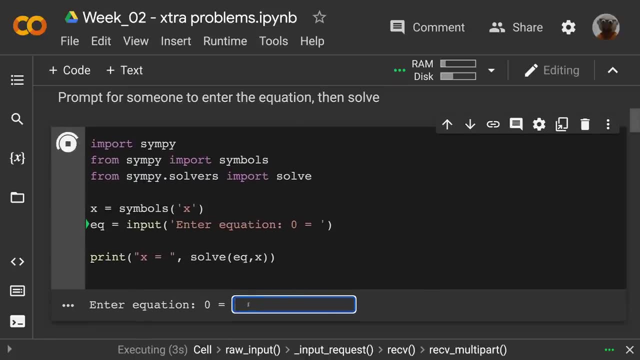 And here then we're solving And just putting that into A print statement. There we go. So we have this. prompts. you enter the equation and maybe I just make it three: X Minus Six. How about that? There we go. 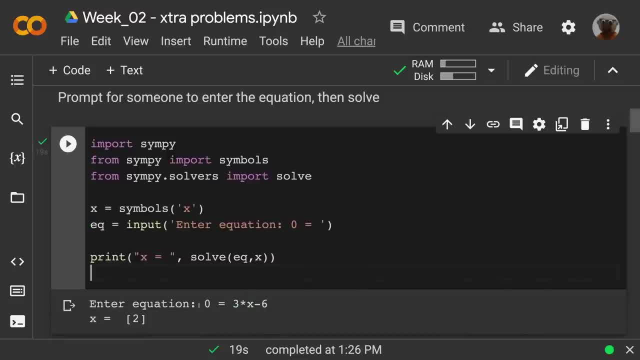 Something good. One solution, Three, X minus six, because if X is two, then that works. Okay, that's great. But again, if you know, I have multiple solutions, or maybe, if I just don't want it to look like this, maybe I want it to be a little bit fancier. 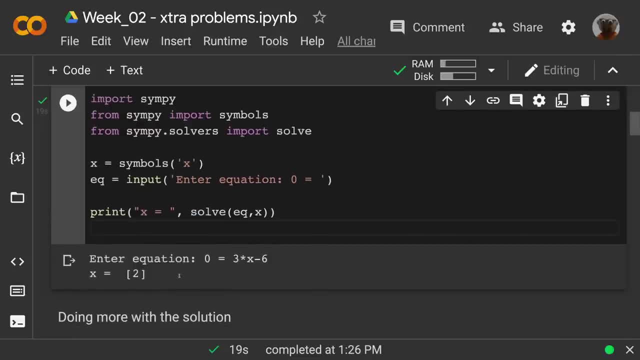 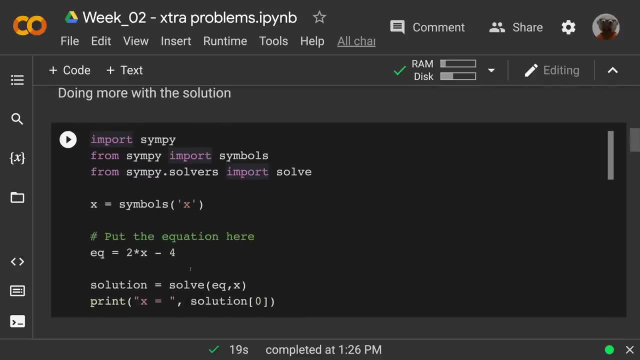 So, again, this solve stores this as a finite set so we can do more. All right, we're going to import all the rest of these now here. knowing that it's a finite set, I'm going to store that answer as this variable called solution. 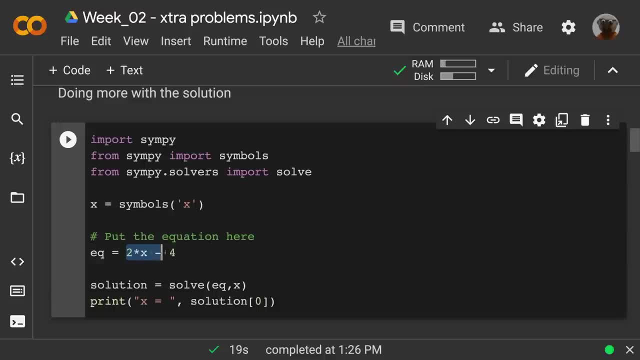 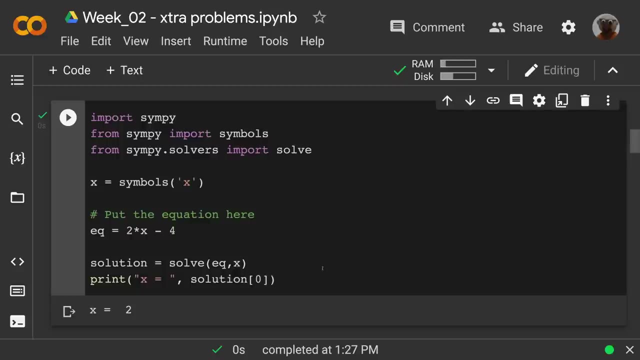 And then This particular equation. I know this has one solution, So I'm just going to have it display: solution index zero. And that's going to be the first solution which, in this case, is going to be the only solution. So when we run it, there we go. 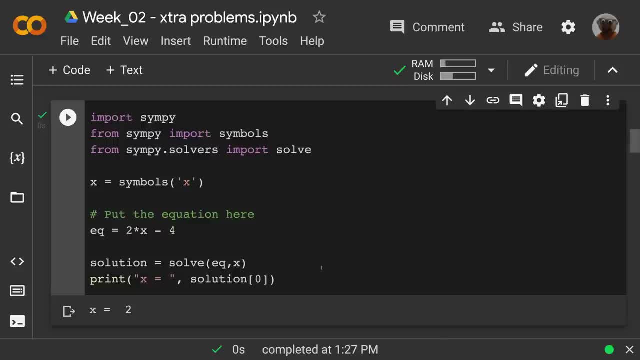 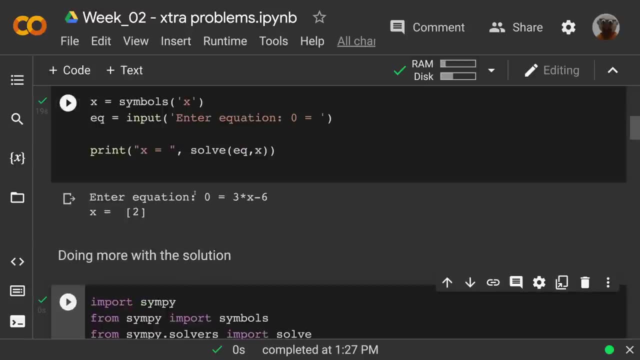 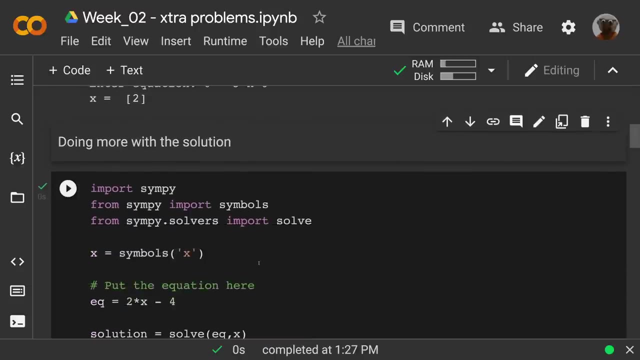 And again, this is pretty useful if I want it a little bit nicer output, just like having that Nice user interface, you know, having it display Zero, Zero equals and then waiting for the prompt. So you know some, some other ways we can do this. 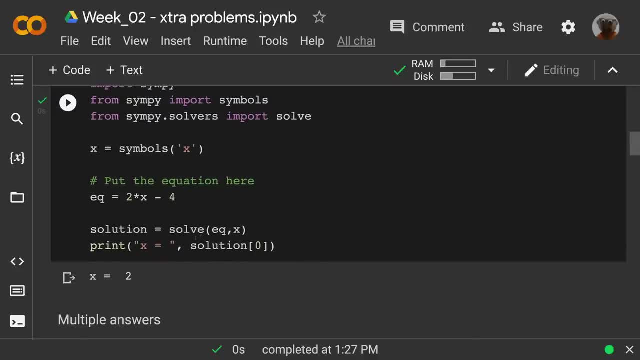 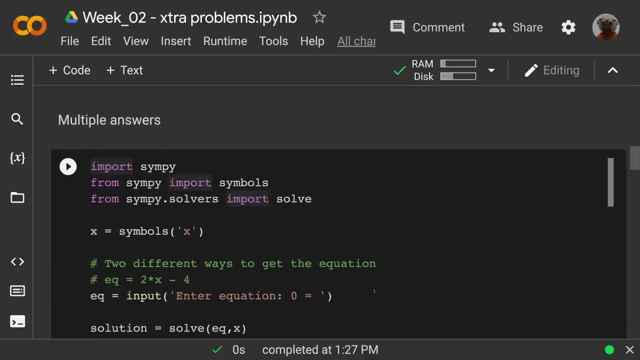 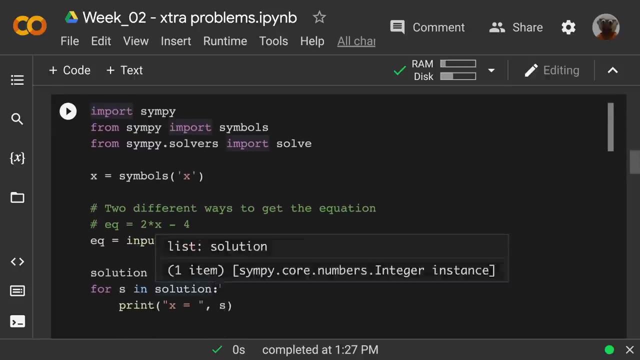 And you know, here's saving this. Okay, that's great. Now what if I have multiple answers? And what if I don't know how many answers I'll have? So I'm going to put this here. So if I enter the solution now, 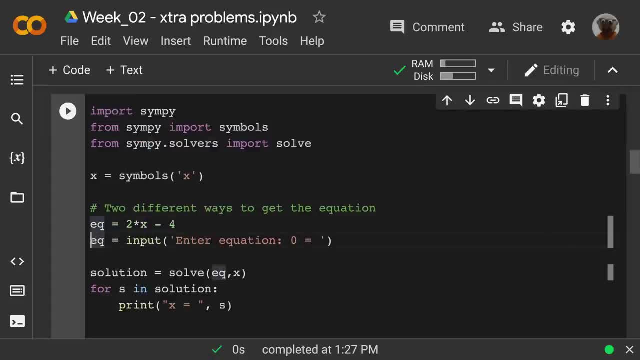 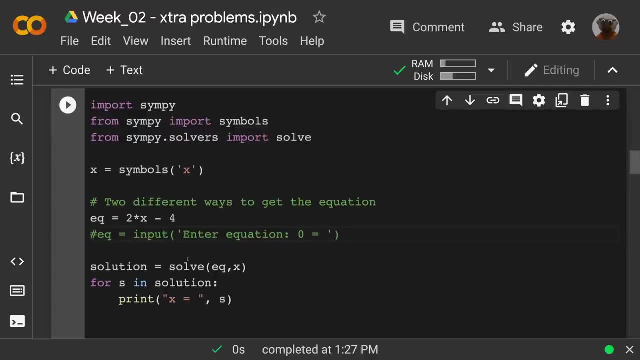 Maybe I'll just Put the first one here. We'll get. we'll get to this one next soon enough, So I'll just take the same solution that I know has one solution And, just like we were doing before, I'm going to solve it and store that as a solution. 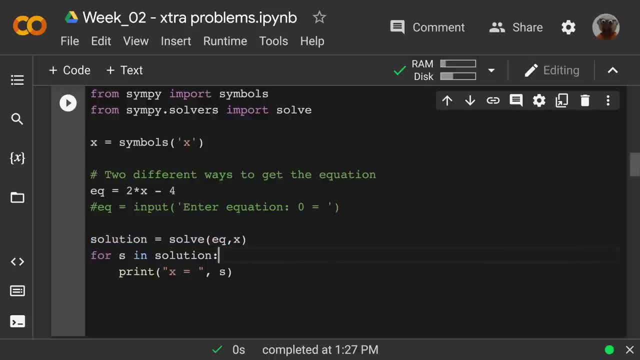 Now notice my loop here. And Python has this great method of iterating through everything in that list. So for S in solution. So there we go. So every item in that solution set, whether it be one, whether it be however many, it'll iterate through that. 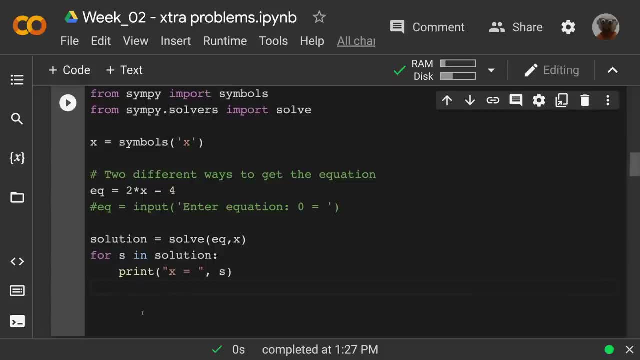 So S is that solution, And then it'll go through, It'll be the next one, the next one, And each time I'm just going to print X- equals, and then I'm going to print out S. So you know, we make use of the Python shortcuts. 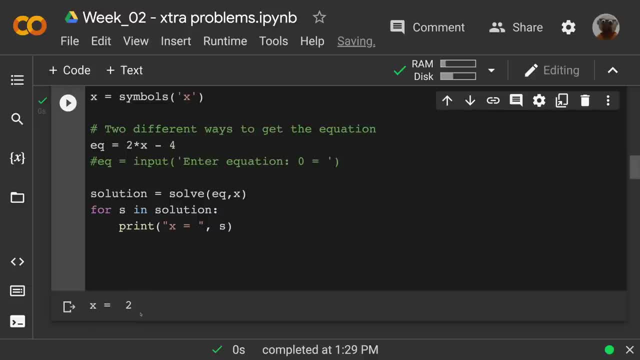 There we go. So Two X minus four, The solution is two, And We went through and did this. So what if I have something like Something that has multiple solutions? And so, And also supposing, I want to Prompt for this- 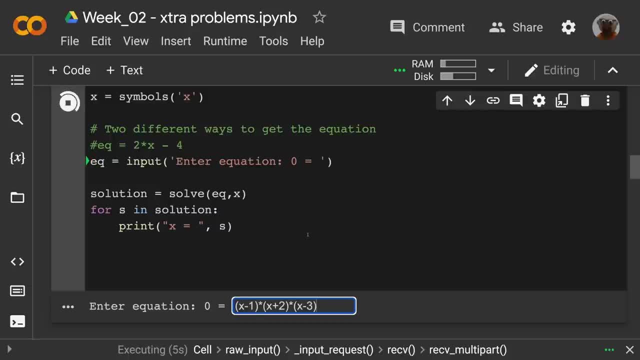 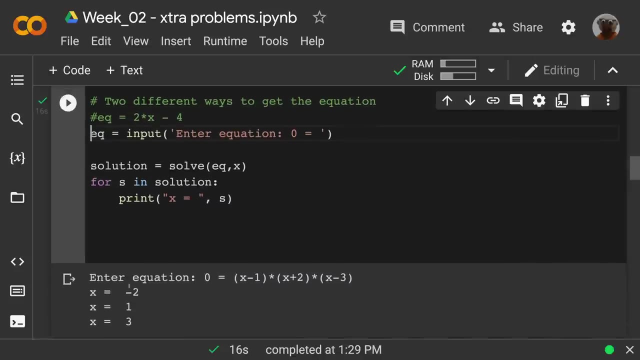 All right. So what if I just plug in something like this: Now, this I know is going to have three solutions, Because the three possibilities that would make that zero. So Let's see what this does. Again loops through and it will output all three solutions. 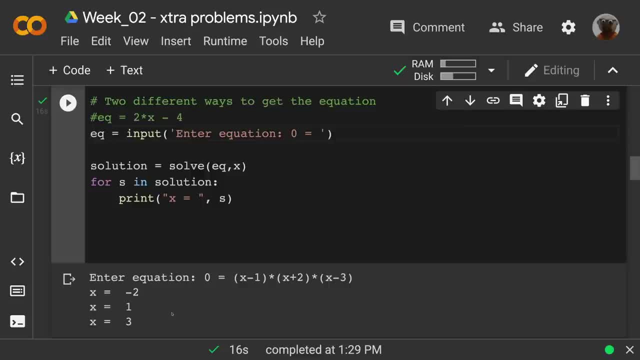 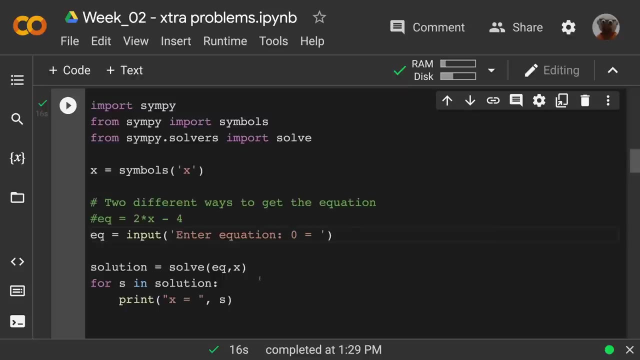 Very nicely. So we see we're building some of these things behind the scenes that will output one or multiple solutions and output it in a nice way. So we see you know, if you're going to copy some code that you're going to use, this is the one to do it. 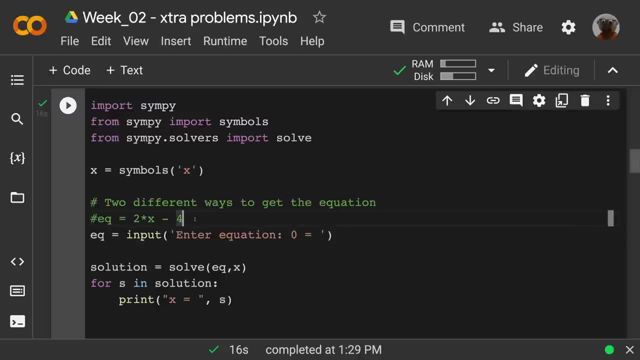 Because you know you could even, like you know, take out this. This was my demonstration, but There we go and You really don't even need these. so this could be your code and That will work for anything, because it's going to prompt anybody- you or you or anybody else- using this to enter the enter the equation. 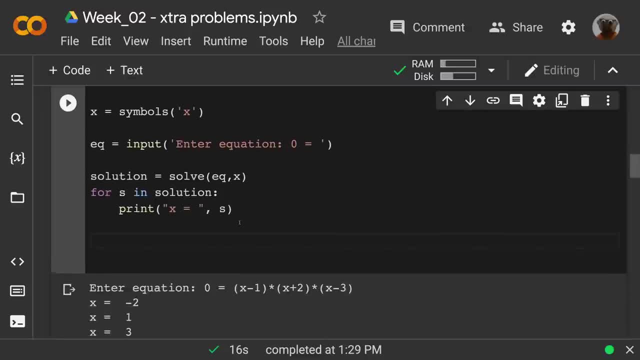 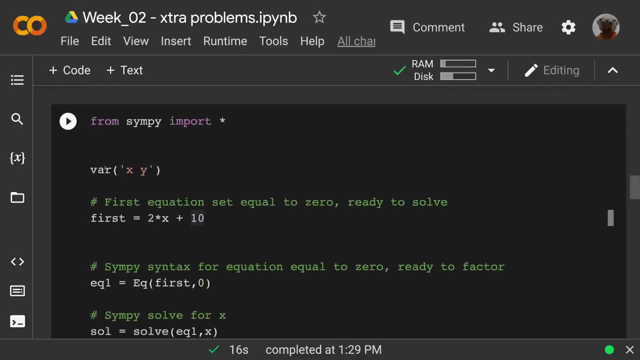 So there you go. You see, we're building some tools here that we can use to solve. All right, What other ways can we do this now? Well, some interesting things were also. this time we're going to call it VAR for variables and we're going to use X, Y, but we'll come back to the Y. 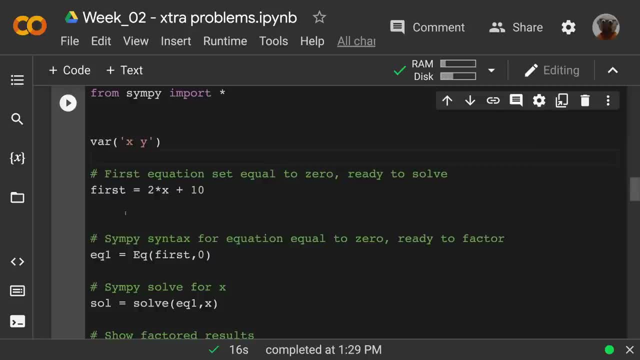 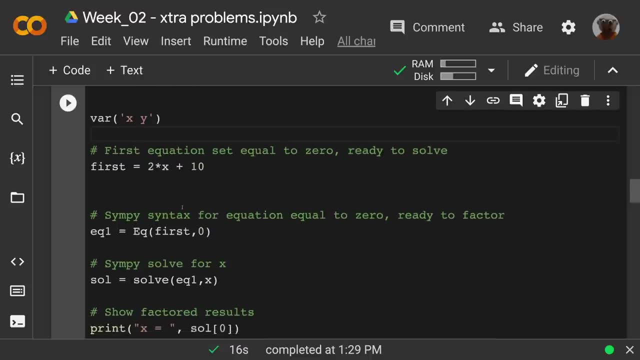 And we have this one first. You can- because you can use this for multiple equations, but I just call this one first. So there you go. Two X plus ten. All right, Now we know that this is set equal to zero. That's kind of the go to way of doing this. 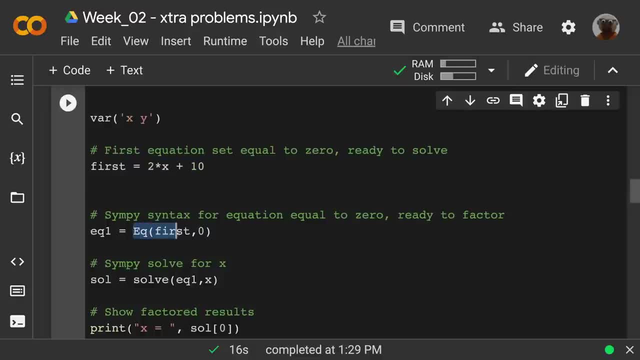 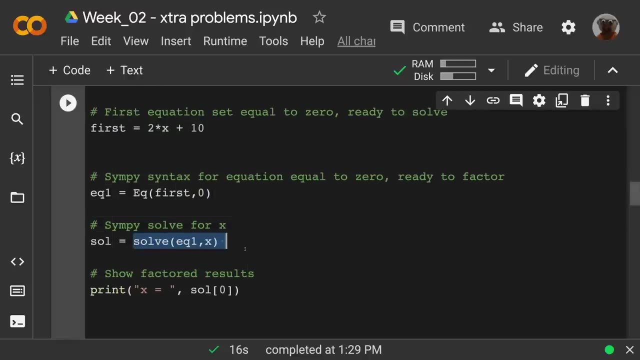 But then this simple syntax, We're actually going to spell it out and define it: EQ, first comma, zero, saying that this is set equal to zero, because then I can solve for X. That's great. And this solution I just called SOL, And since I have this one, I know that the solution is. you know, there's only one. 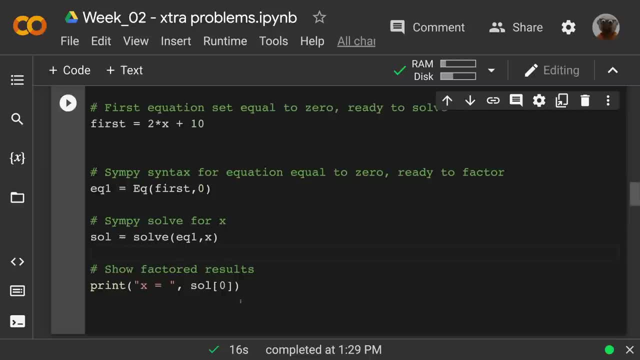 So I just put salt. You know that's my finite set And I want the first Index, zero. So this is it, And actually these are factored results. But this is actually going to give me a nice actual answer, because I can get that answer. 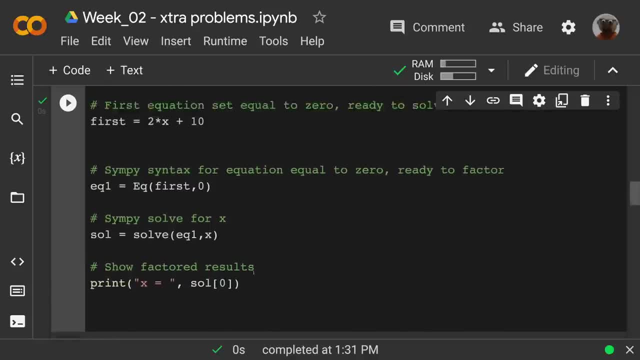 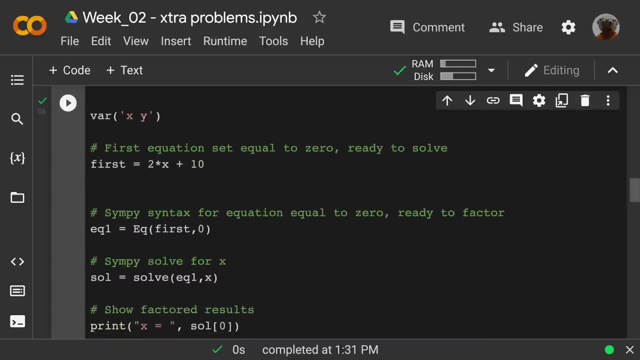 X is negative five. All right, Now here's where Y comes in. Now I have to have Y there. If I define Y as a variable, Now down here I can say: supposing this is equal to Y, And you see, that works. so spelling it out here that it's the equal to Y. but now I now I'll solve for X. 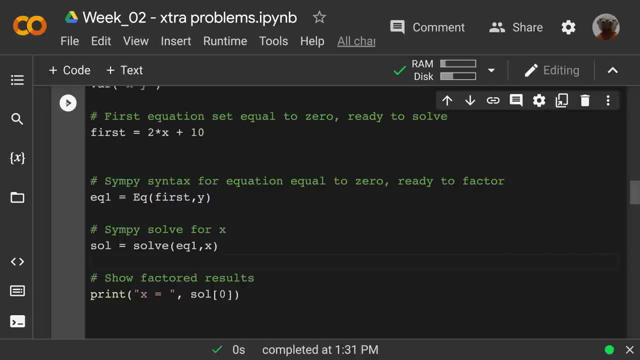 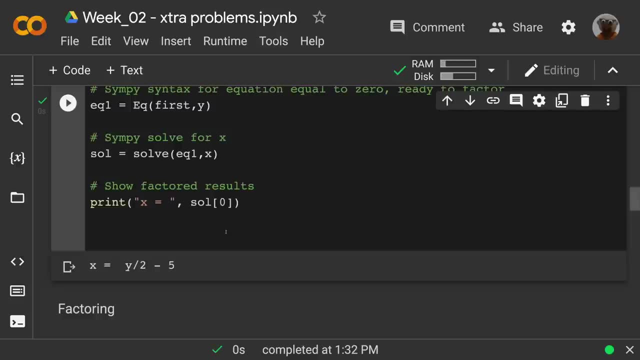 So that's kind of interesting. And then when we do this, you see Python could actually do some of this factoring for you. you know rearranging an equation algebraically. So now it's solved: Y over two minus five- Pretty cool. 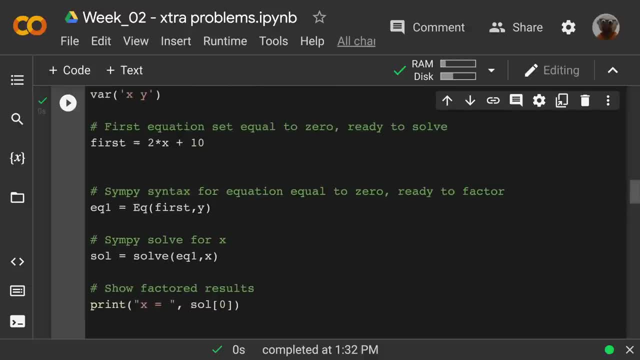 So we can do some things like that, We can rearrange things And then if I have this, You know I could, I could change it around a little bit or whatever, but some, some different things you can do. The default is: make this equal to zero. make this equal to zero. 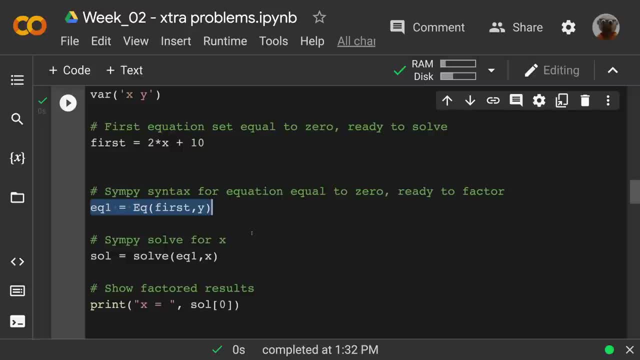 But this gives you this other flexibility: You can call it equal to Y And then you can do some other things, You can solve for it. So, pretty cool. As you do this, as you incorporate this into you know, some of the notebooks that you're going to create tinker around with this and, you know, try some different things. 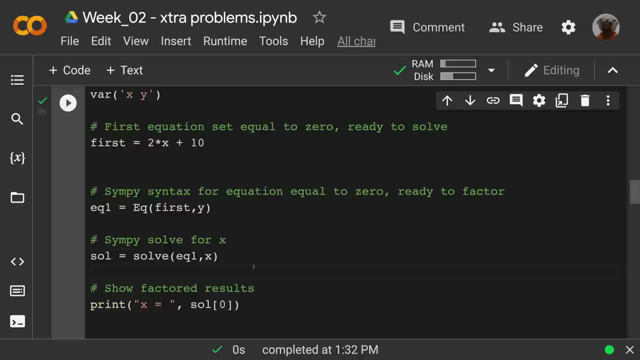 You know that's the idea. We go through some different, some different formulas or different equations in a textbook and say, hey, can I try this? Like we could take a look at this and say, all right, let's see. solve for Y. 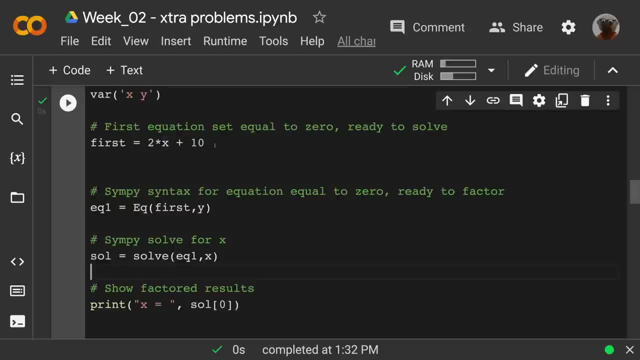 Now what about? if I have Two X, then then if, if, if I want to solve it for, and you can even include Y in here, So there we go, And if that's included in Y, then I still might then go back down here and say that this is equal to zero, because that's kind of the default way for that to go. 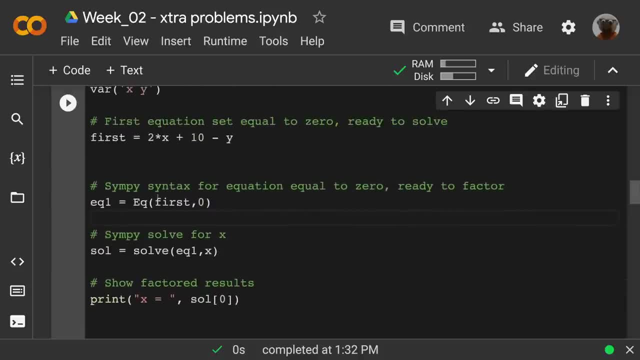 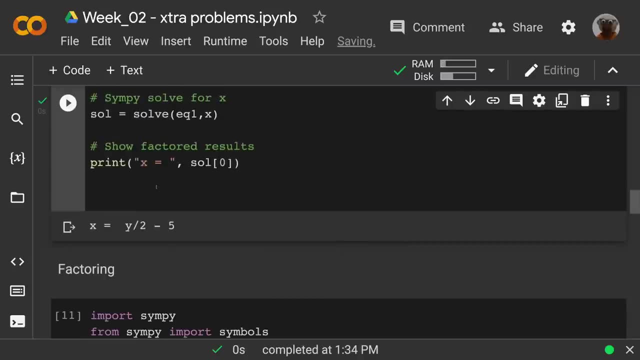 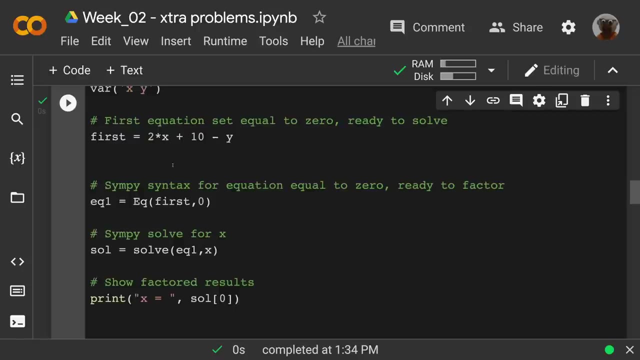 And I I can still go back and solve For X and it should end up being very similar, because whether that was, you know, without this minus Y saying it's equal to Y, or with this minus Y saying it's equal to zero, 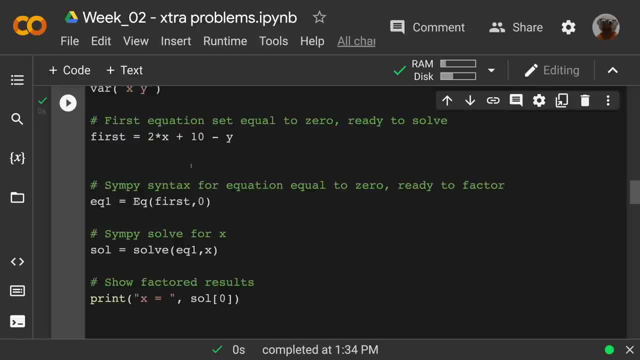 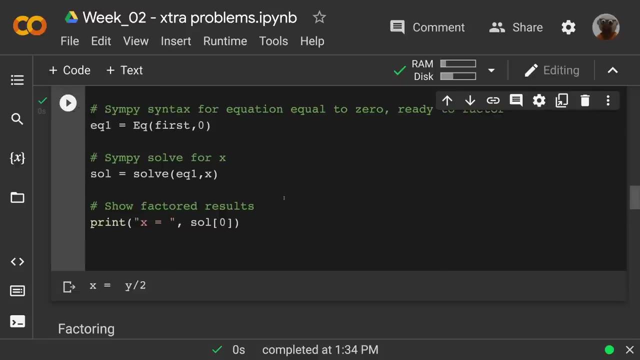 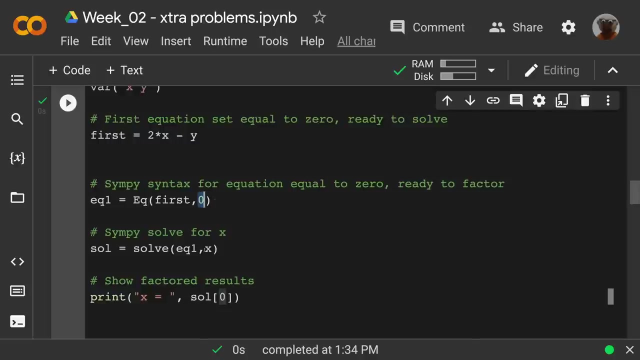 See, algebraically very similar, And you know, we could even, just to show you, we can even say this to X minus Y and we can run this. There we go: X is Y over two, all kinds of different things you can do. if you need to rearrange this, you can put that in this set up here, and then you know what is. what is this set equal to now and what am I solving for here? 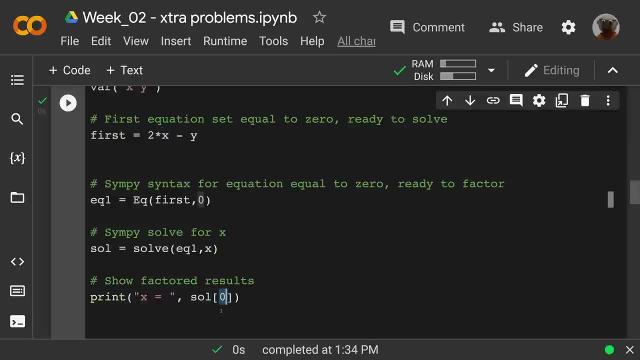 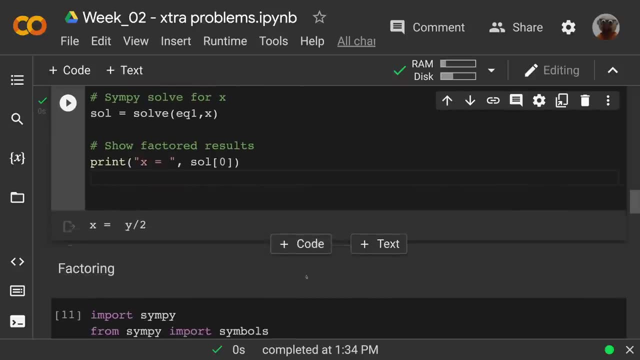 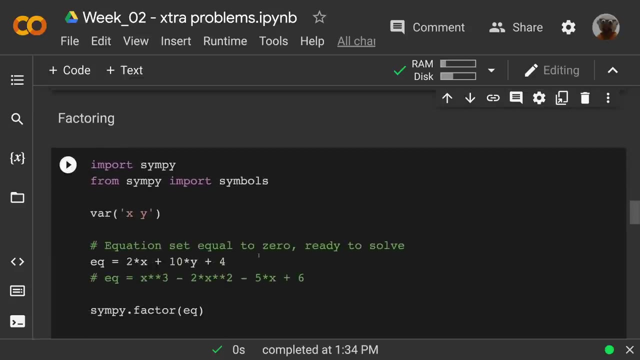 And in this case it pretty much will be index zero for that solution set each time. So these are some cool things. you can get the code to do all the factoring for you. Well, here's some other factoring. Supposing I have something like this: you know we can divide out common factors. 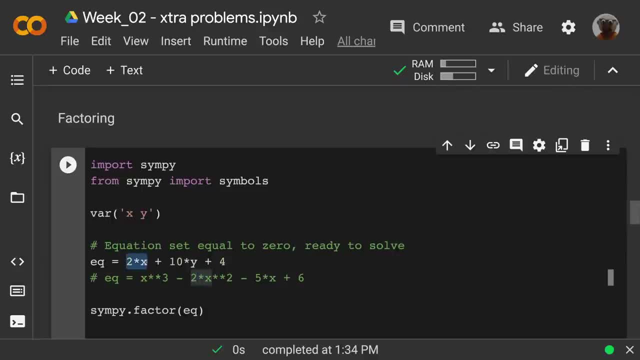 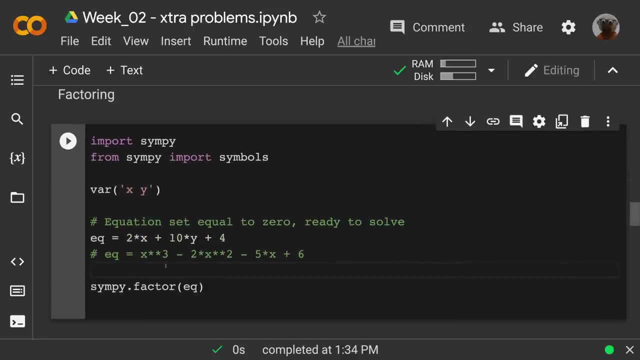 Now you might see this: two X, two times X, 10 times Y plus four. Now, supposing this is another thing, in simple I can just factor it. You know I'm not saying that's equal to zero or anything. 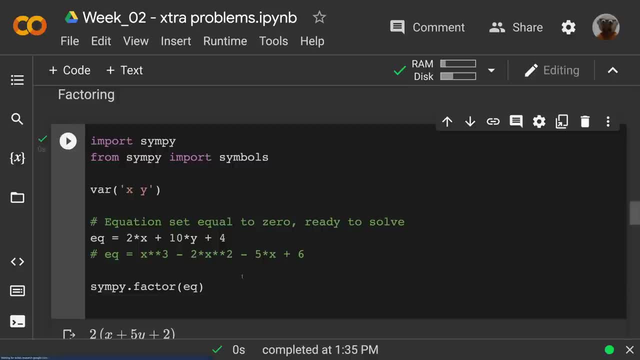 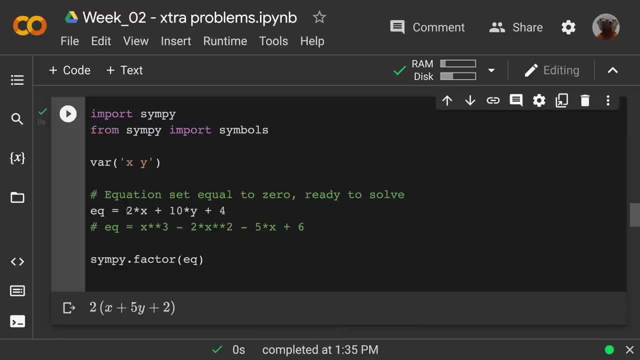 I just want to take a look at this and I want to factor. Look at that And simply also does the nice display on the output too. So you see, there was a common factor of two And that worked. Now, supposing I had this, and let's say this is three, which then doesn't factor at all. 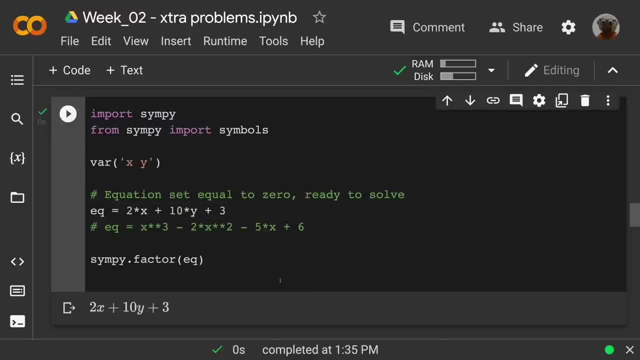 So when I run it, You know it will just output that because it's not factorable. All right, Now What's really interesting is if I have something else like X squared, And let's say X squared minus four. Now 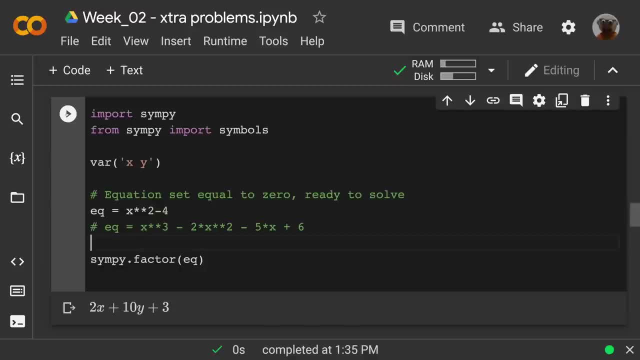 You may or may not be familiar with that factoring, but I can factor something like that too. I look at that. It'll factor that out. That's, that's the correct factoring of that X minus two, X plus two. So it will do a lot of really interesting factoring for you. 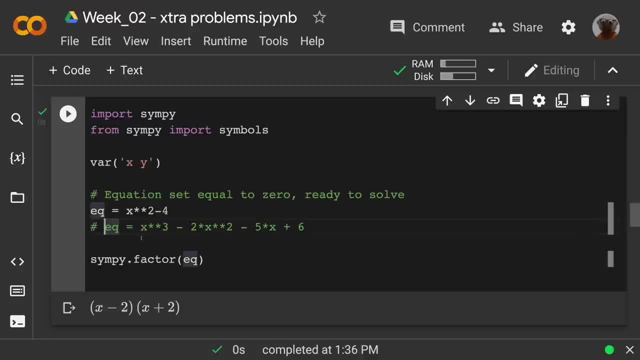 So pretty good. Here's another one that We can, you know, just to show you that we can even take it to the next level: X to the third minus two, X squared minus five, X plus six. So we have that, And if I factor that, 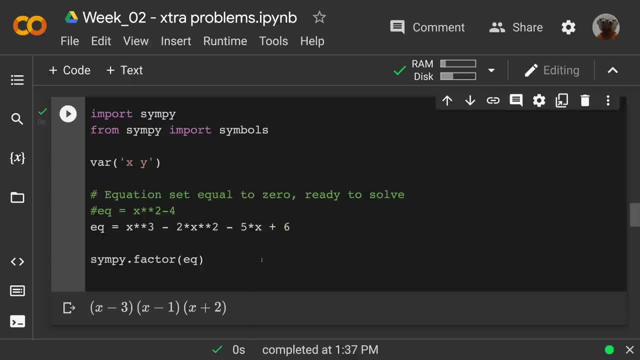 There we go. Look at that. It breaks it down into Into, into these factors. So some of these really good things you know, knowing that you can set your Factoring calculate, you can make your own factoring calculator here. 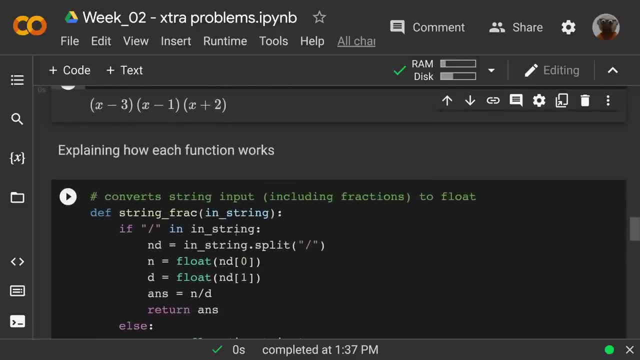 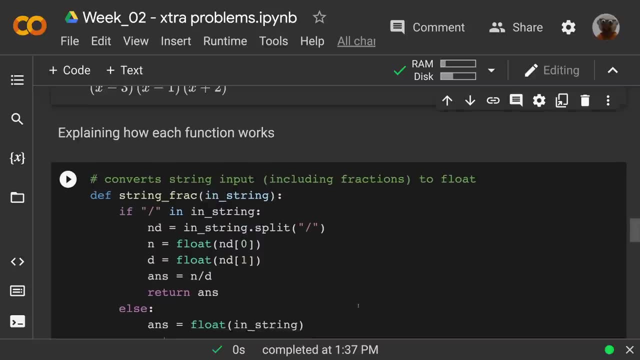 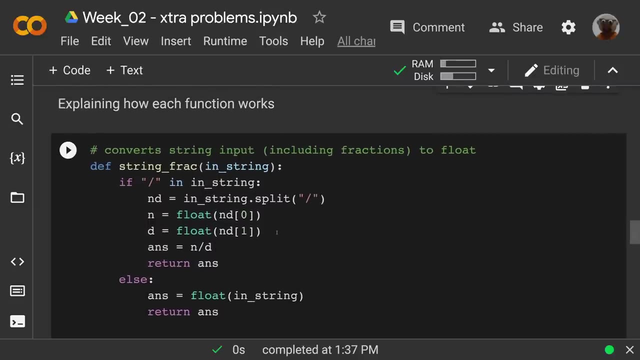 All right. So Let's take a look at some of the functions here. So when we have- you know we have that we can factor, and then you've been doing some of this practice with these functions, So I want to show you, you know, looking at these. 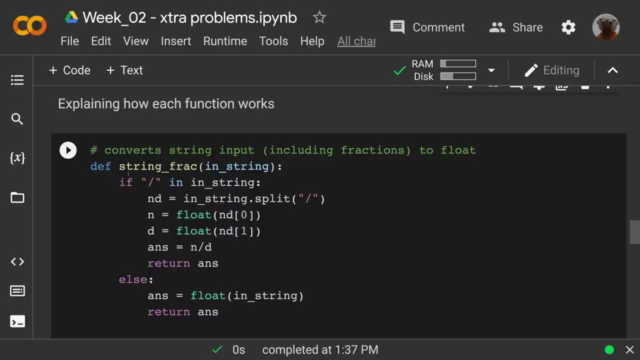 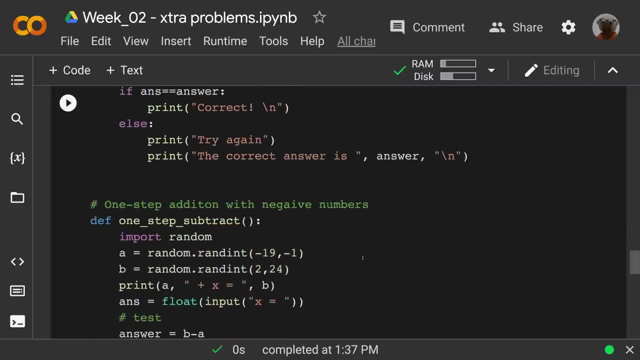 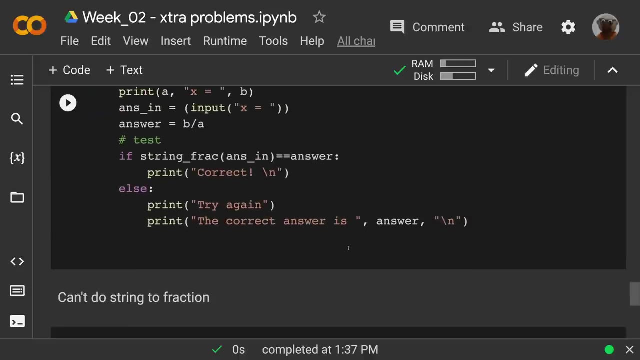 And there's a different input: how we can, how these functions are working, that you know- remember you were doing the practicing- the one step functions, Um, the one step addition, one step multiply. there we go. Now. that first one I want to show you is because you can't do string to a fraction. 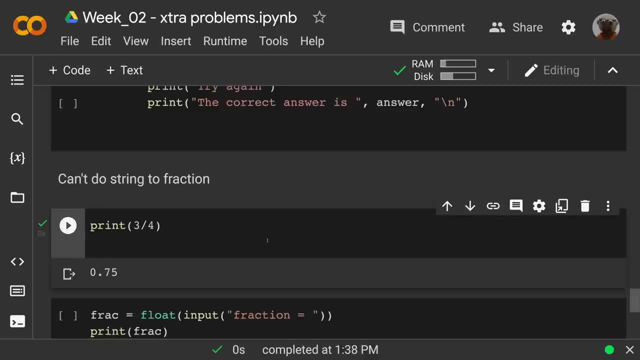 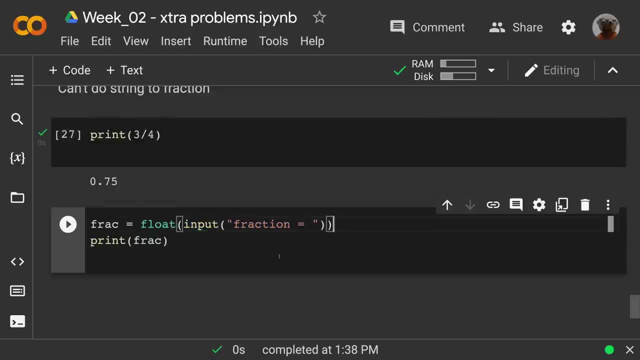 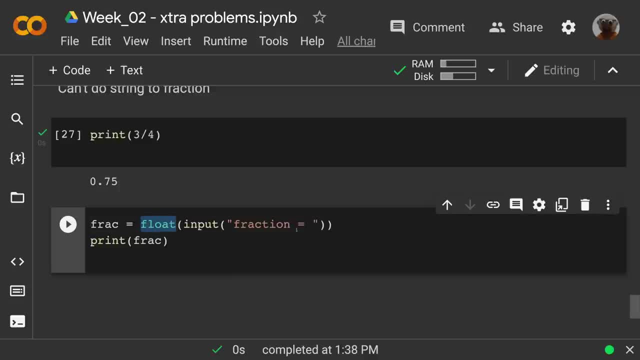 So that's a number that could include a decimal, but if you know that it's going to be a fraction, this float won't work because that slash for the fraction doesn't parse nicely. So then this will give an error. now, just because it. 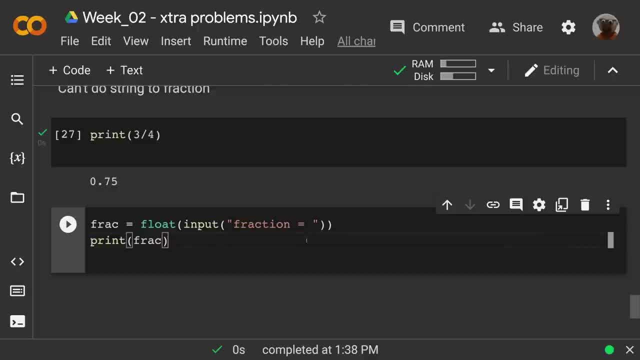 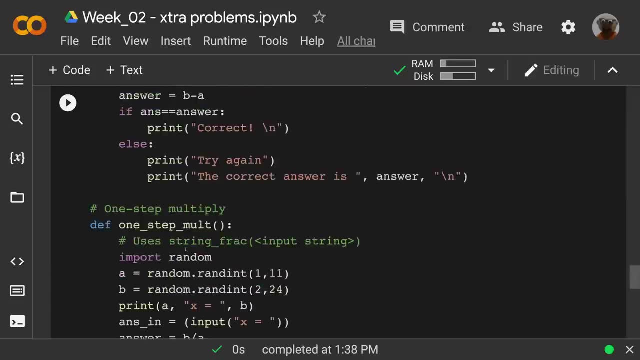 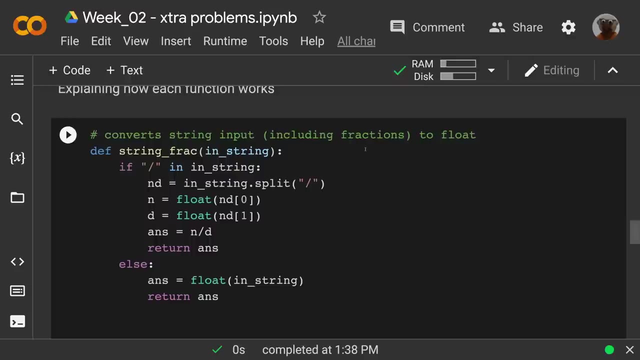 Says fraction here. That's just a display. If I just disobeyed that and put in a number, then it wouldn't give me an error. But if I, as soon as they use that divided by, I need that. So that's our first function. here is: how do I convert the string input, including fractions, to a float? 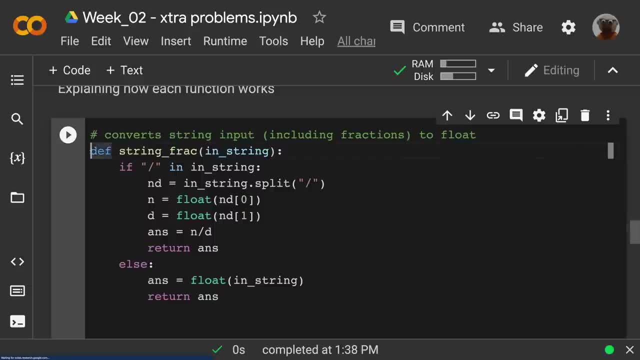 So this is the way Python functions work. I'm going to use this D, E, F to define it And then, once I define that function, Um, I give it the name of the function. I need the open and closed parentheses, and this particular one will also have input. 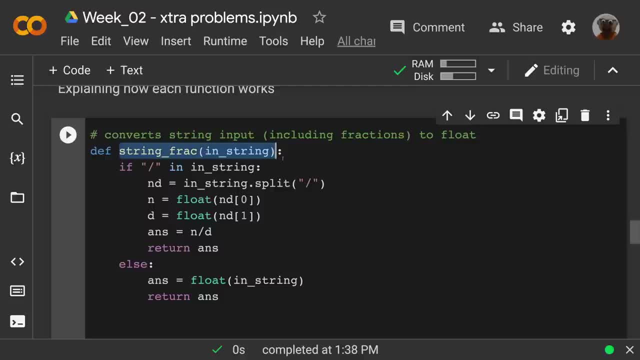 So I define this variable in the parentheses. That's going to be the input and then colon at the end. So once I define that, then everything under this is indented for spaces. Yep, And I recommend: don't use tabs, use indentations. 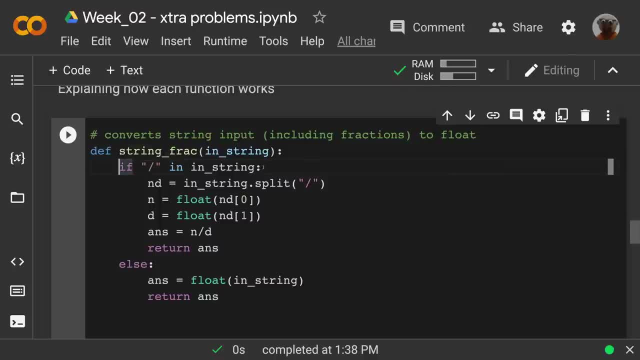 So then I have an if statement and if, and then here's the condition: if this is true, colon, and then that's indented for spaces. Okay, So I take this input string and I'm testing to see if this fraction bar is in there and notice if this exact character in in string. 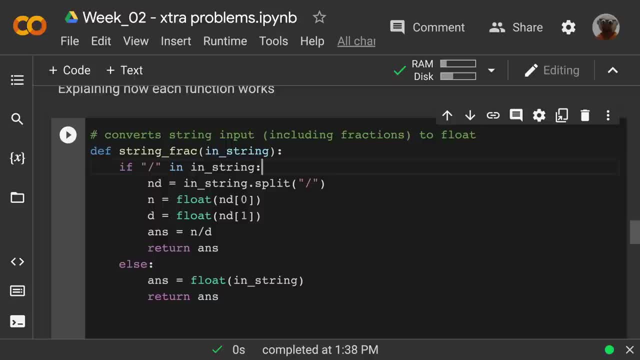 Cause. that's what I called it, That's my input. If it's in there, then we have this split. Each string has this split function, So you can split it and say, all right, at this point I'm going to split it. 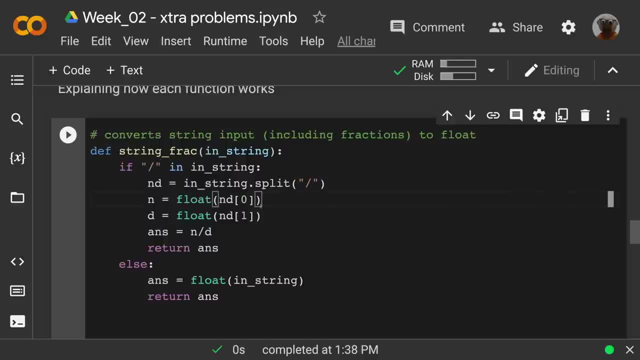 And then that creates two different arrays. Now, this was all based on string input, So it's going to be two string arrays, um, or two, or one array with two elements, And so it's going to be Nd. I call that for numerator denominator. 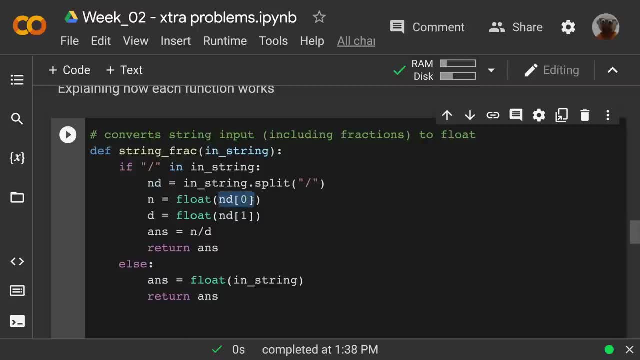 So then Nd0 is going to be everything before that And Nd1 is going to be everything after that. So if this was a fraction, if somebody put a fraction in there, then Nd0, everything before that would be the numerator. So I'll cast it as a float, store it as N for the numerator. 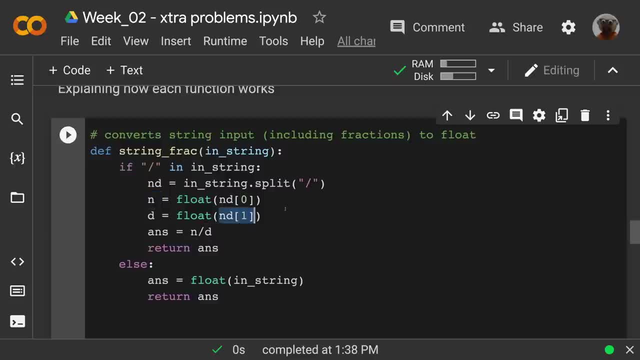 And then nd1 is everything after that. so I will cast it as a float, store it as d for denominator And now see, we had to split, we had to detect that, split that string and then each of these two elements individually, cast them as float numbers. 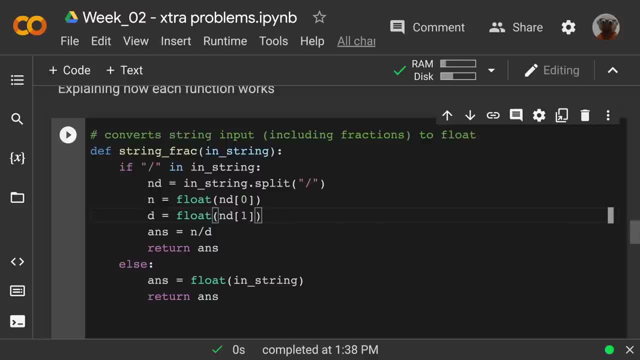 and now these are numbers n and d, and now I can actually do that division n divided by d. So you see, because that slash doesn't work for parsing numbers, I have to work around it, and now I have ans as this answer. 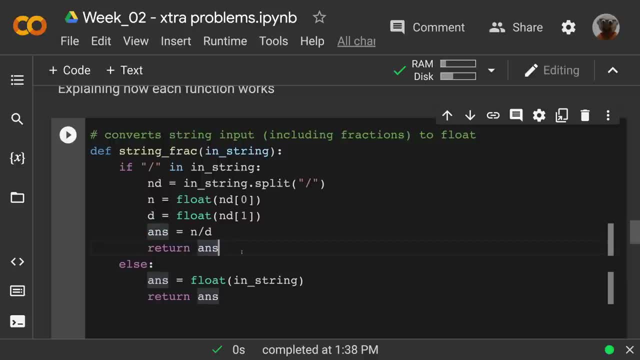 And then I have the return statement. so this function doesn't have a print statement, it just returns this and we'll see how that comes out, but it just you know. wherever this function is, it'll put that answer. So that's if it has that and if it doesn't. 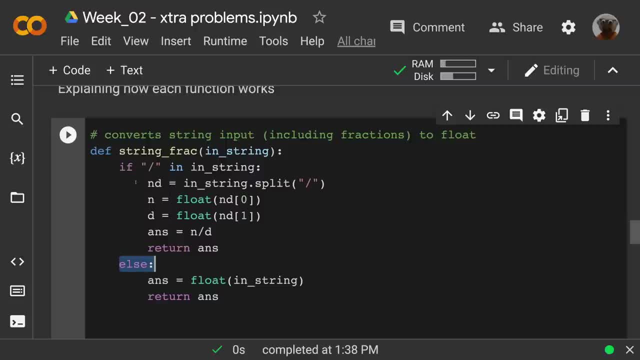 because I want to use this either way. so anything else colon indent, then I won't have a problem. so I'll just take that in string and cast it as a float. That works. So anything else we put in, we're good. 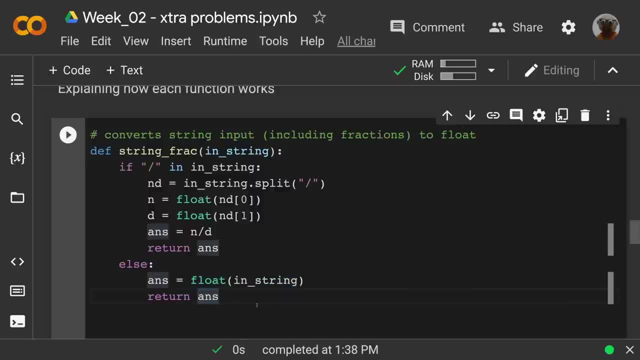 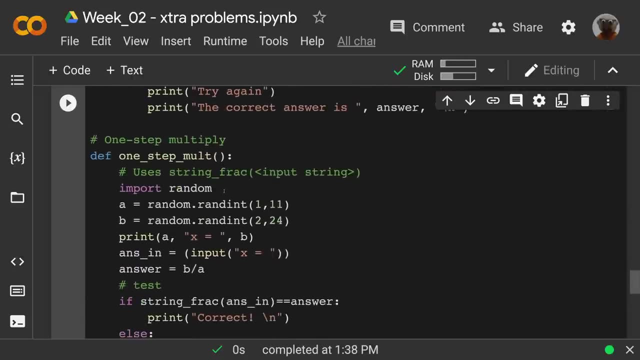 And then again return ans. Now where this comes in, I'll come back to that. one is in the 1.. So here's this function, one step, and I put this common in here to remind myself or anybody else using this that it uses this function. 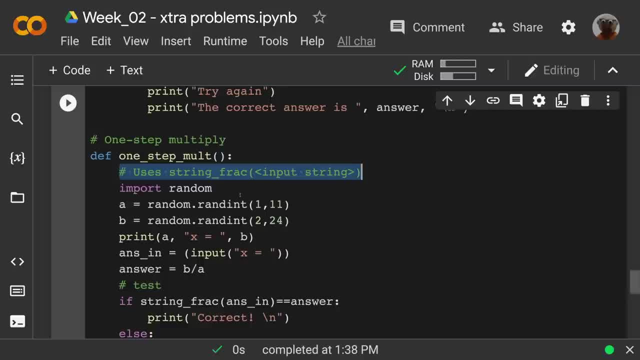 so we need to make sure that it's in the same place. All right, so here's what I did to generate, you know, some practice problems for you: Import random and then here I'm going to get randomrandint from 1 to 11.. 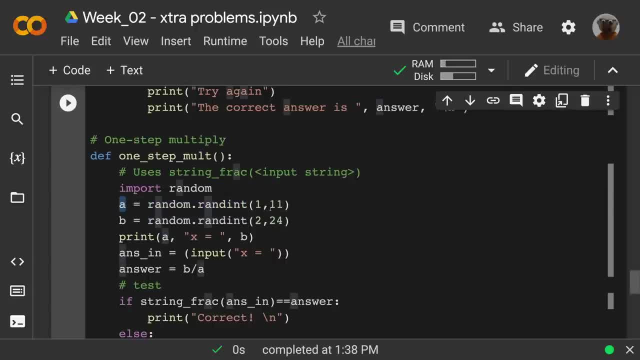 So here's what I did to generate some practice problems for you. So that's going to be a random integer and I'll store it as variable A. So that's going to be a random integer including 1, but not including 11.. 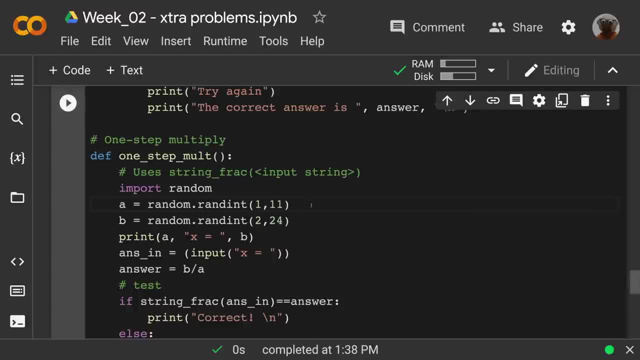 So 1 could show up, 10 could show up, but 11 won't. So that's the way the random integer works. It includes the first one, but not the last, And then B- I just wanted to make this- 2 to 24.. 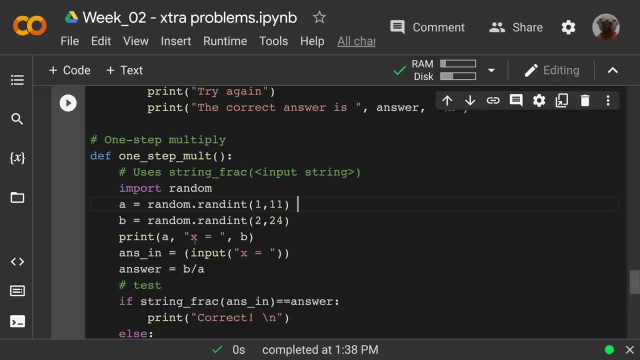 So, given these two random integers, notice what we're going to print here. So AX equals B, So we see it's always going to be something times X and I just want to display this so I didn't need to worry about the Python syntax. 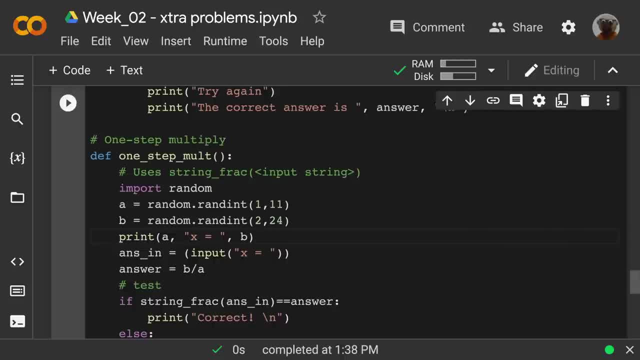 to show the multiplying. All right, so AX equals B, and then you would know what do you want to do? You want to divide both sides by A. So you know that and we're going to take your answer. input. 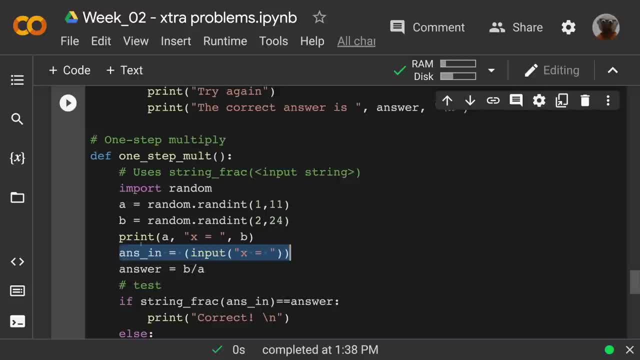 you know, X equals and, whatever your input is, we'll store it as ans in. And then the actual answer at this point is going to be: we know, divide both sides by A. so the actual answer is going to be B divided by A. 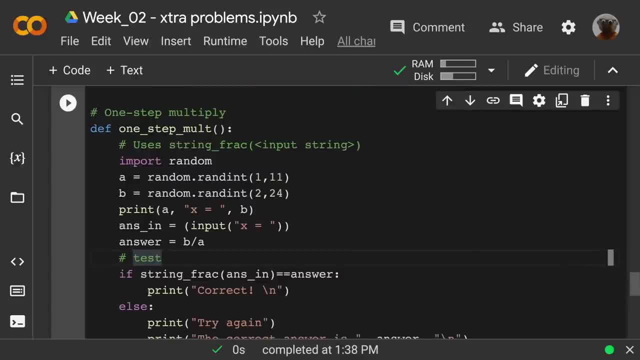 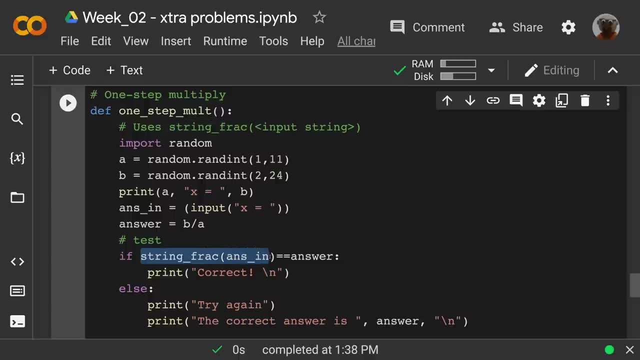 So then, this was the actual input. Notice it's still a string and that's where we're going to use that. We're going to use that in our function that we created earlier, string frac. So see, it's going to take that answer. run it through that function. 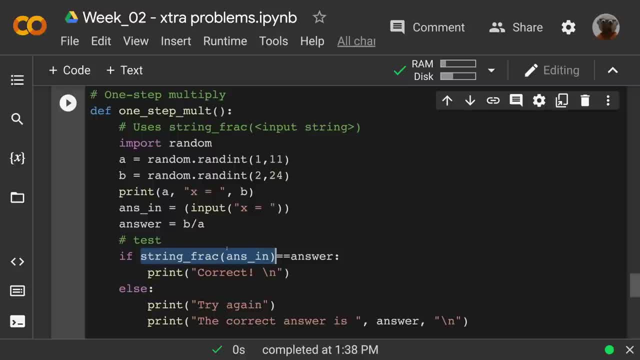 and return right here that answer, So that way we can easily compare it, because this function will return that answer and then the double equal sign to compare, and we're going to compare it to the actual answer. So there we go. So that's the return statement. 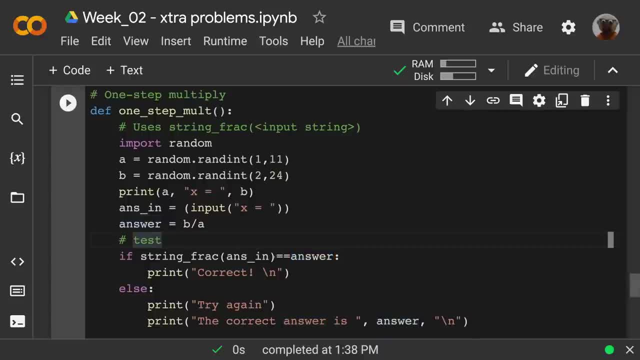 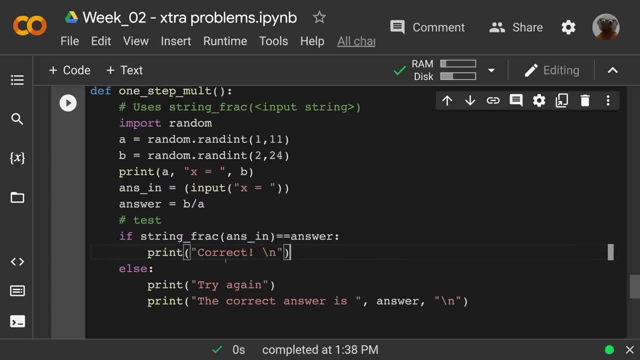 I don't have to. I don't have to print or output anything. It just returns that value right here where I have the function, And if it is good, we're going to print correct. If not, try again, but then print out the answer. 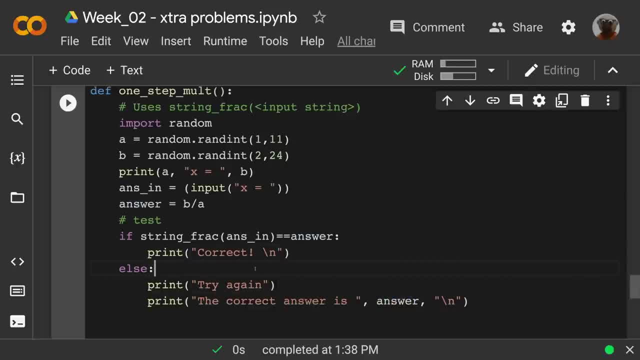 So there we go, And now it'll loop through this. Well, this will do it once, and then you know, we can create a loop to have as many of these as you want: Practice one-step equations. So there we go. 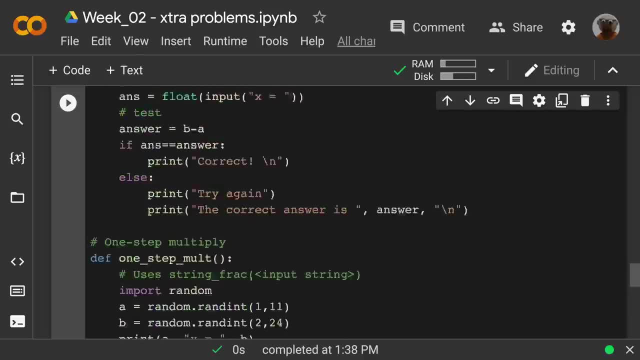 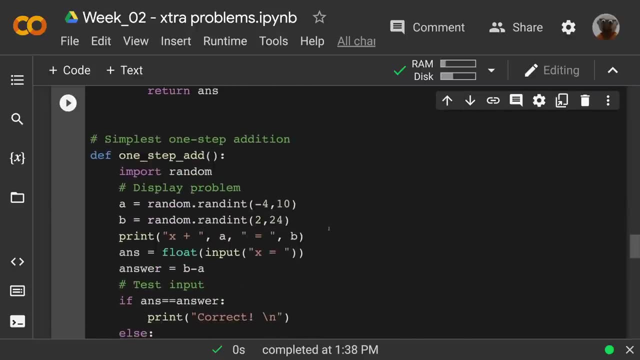 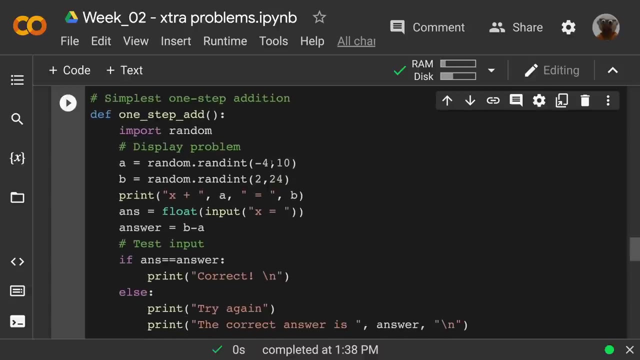 There we go And then test them each time. So you know we have the simplest one-step addition is another very similar one. There we go: Import, random Display the problem, Random integers, And, yes, you can go through negative numbers if you want. 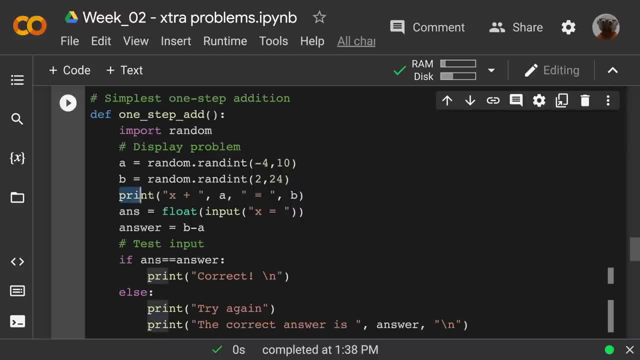 All right, And what are we printing out here? X plus A equals B, Because then you know that to solve for X subtract A. So we'll take your input. What do you think X equals? But also, we're going to calculate exactly B minus A. 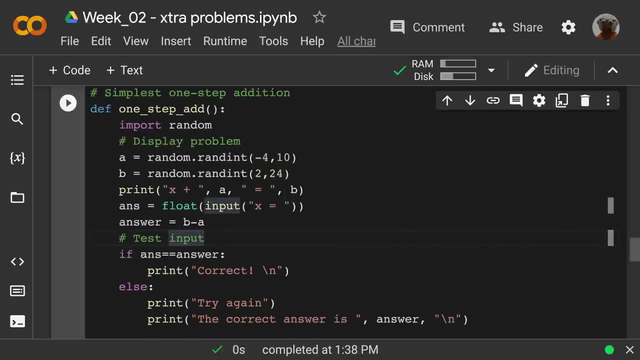 What is it really? And then down here, we don't need to do anything else, We just say: if A and S equals, answer. There we go And here see, we can cast the float. We can cast the input as a float right away, because we're not expecting anything fancy. 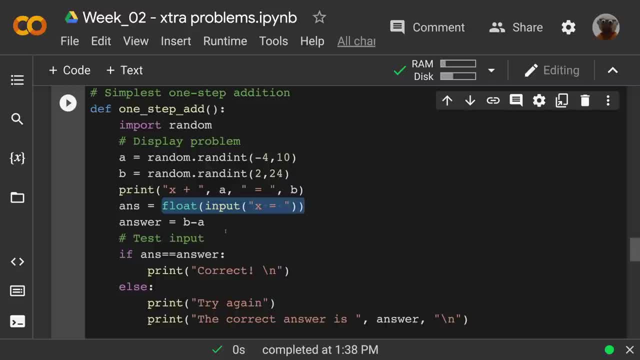 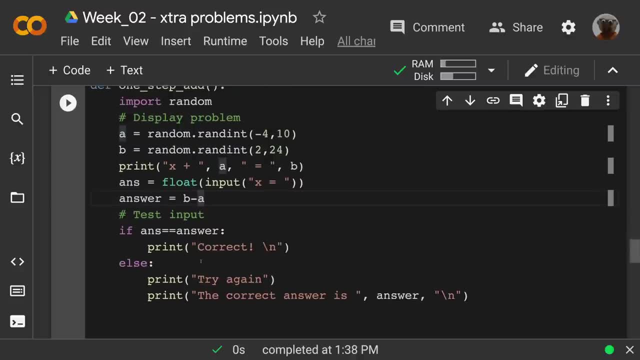 You see, the other one, Knowing that I'm going to divide. you know I need to address all the other things that could come up. And there we go. If it's correct, there we go, If not, and then we print out the answer. 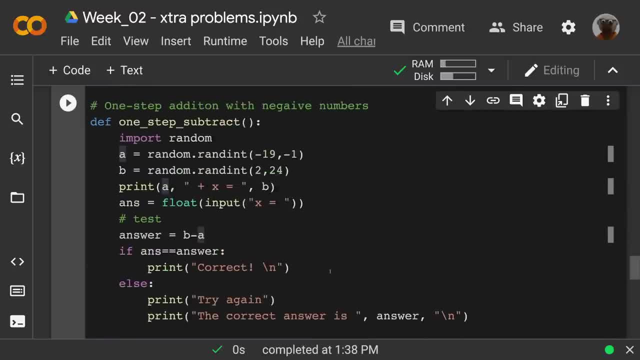 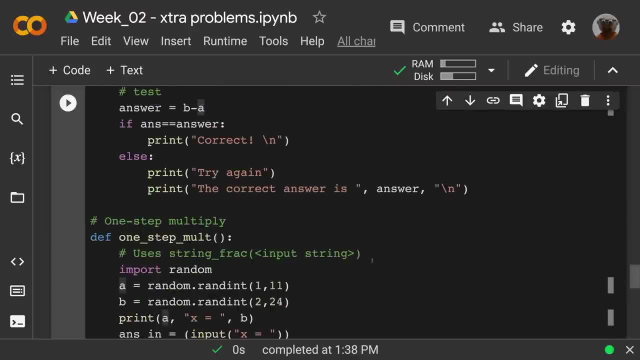 Cool. So some different things you can do. And you know one-step addition with negative numbers. Just We just did it in a slightly different way. So here's a bunch of things that we can do, Just practicing your own ability to solve. 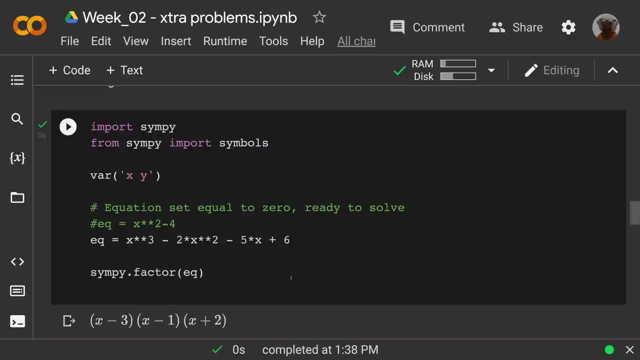 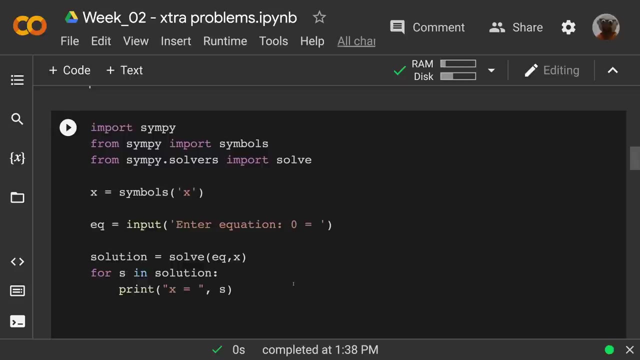 We'll also get more into some other functions later, But you know good to see these functions. But yeah, yeah, here we go. Just some of the things you can do: Factor or solve. So these are the things that you want to be able to do. 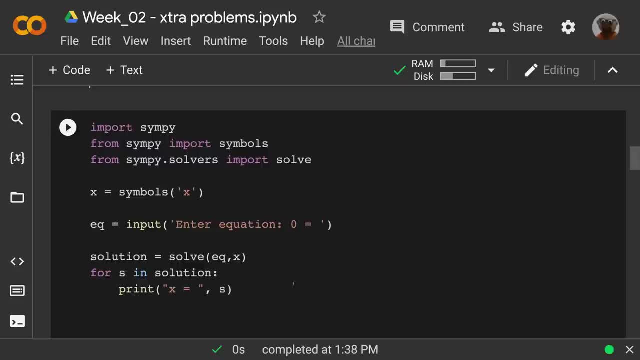 And you know set up, you know start again, start building your own, your own Colab notebook. So by now you might have some things that you know solve for proportions. You might have some things to you know solve for X. 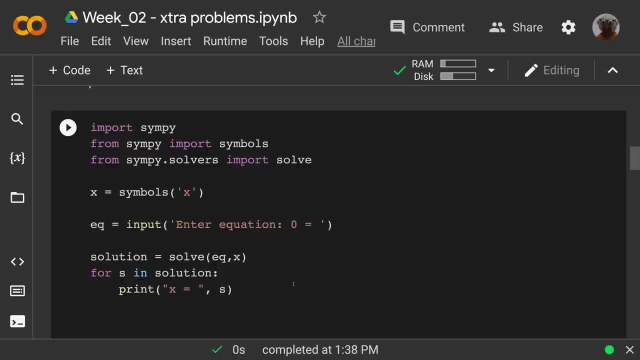 And you know, maybe you can even copy one of those you know, convert fraction input to something You know. feel free to. you know, copy, copy these, tweak them, make use of them on your own And you know. you see, you're building your library as well as really understanding the code as you're building this. 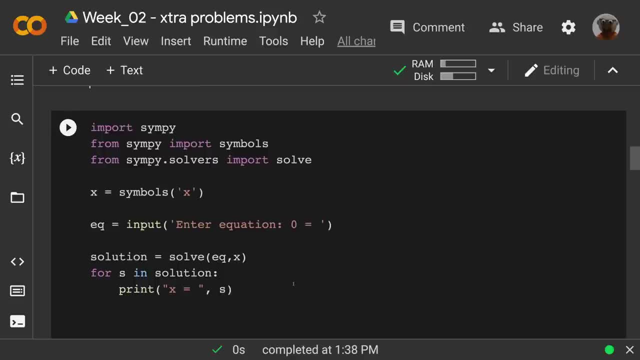 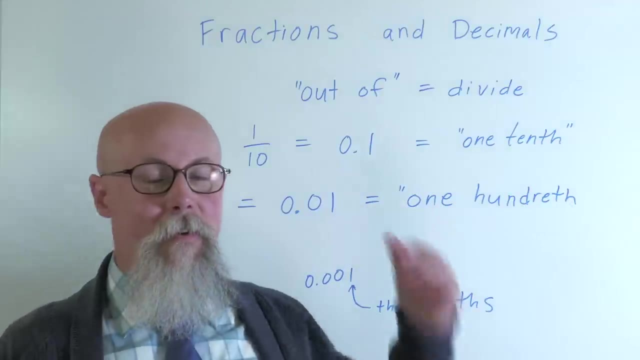 And you know, hopefully your understanding of the math and understanding of the code gets deeper and deeper as we go on here. All right, So I think we're ready to go on to the next unit, So let's talk about fractions and decimals. 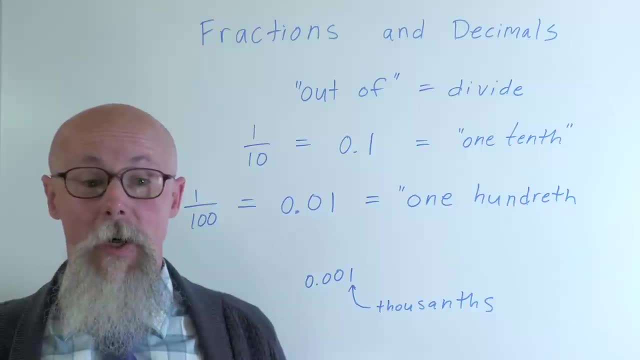 And how to convert from one to the other. Well, fractions, when I say out of, like, this could be one out of 10, if I say out of, that means divide, So any fraction numerator divided by denominator. you can do that on your calculator and it most likely is going to return your decimal. 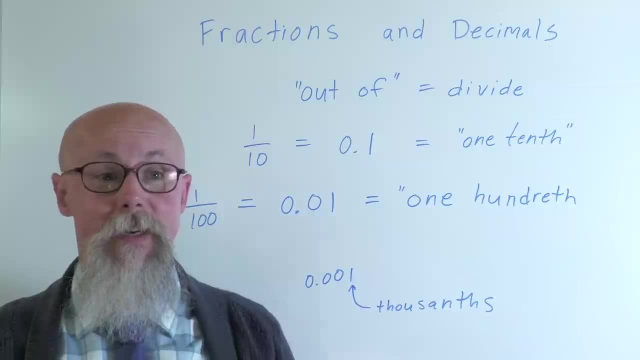 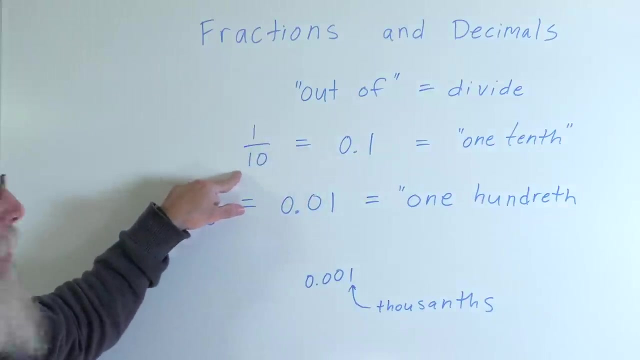 There you go. So fractions, decimals, you know pretty easy calculator. do the division and then you know you have your decimal. but what about doing it in the reverse? So when we look at this, this, I would read each of these one out of 10, I could call it one 10th or 0.1 is what you would get if you did that division. 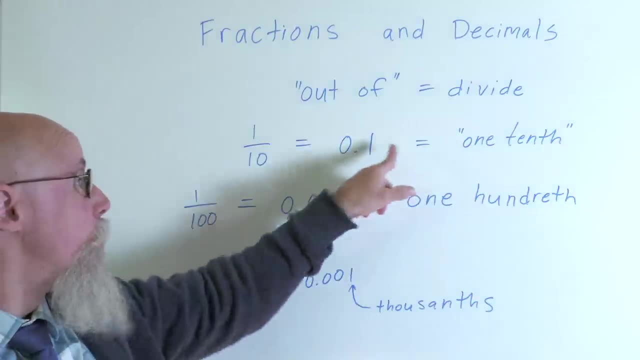 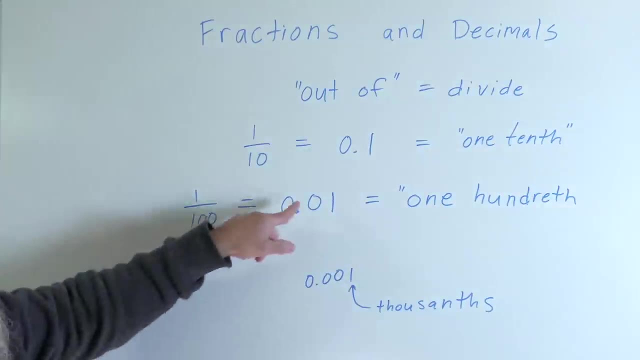 I would still call that one 10th, because that first decimal place is the 10ths, So that would be one 10th. Or then if I had one out of a hundred, then there we go, Two decimal places So 10ths. the second one's the hundredths. 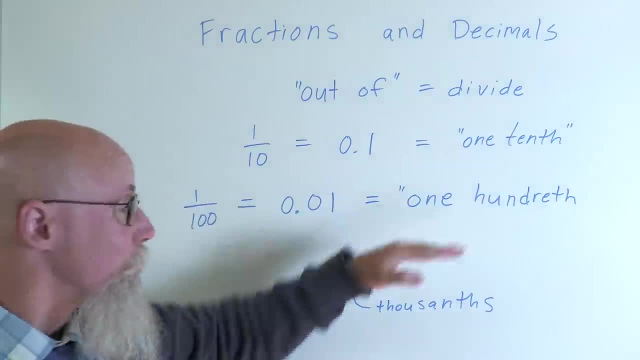 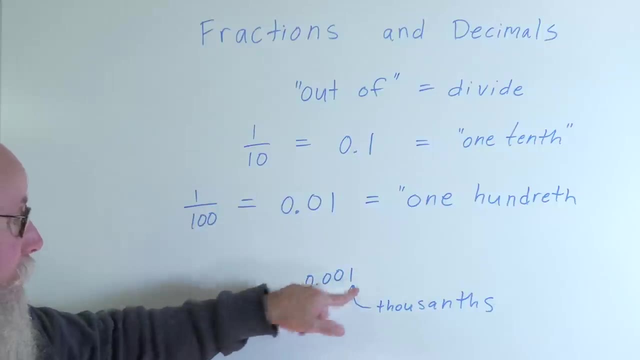 So whether I, If I were to write it like this or like this, I would still call it one hundredth with the TH. Then, you know, I just wrote it one more. you know, third decimal place would be thousandths. 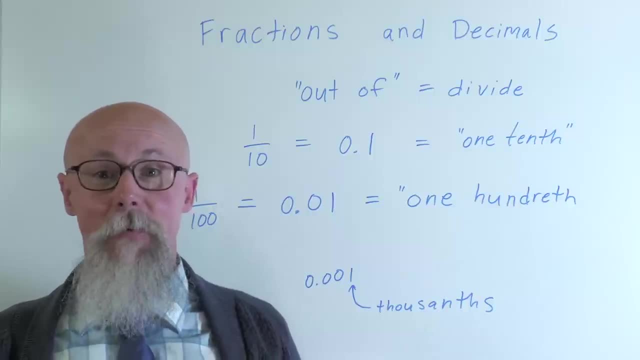 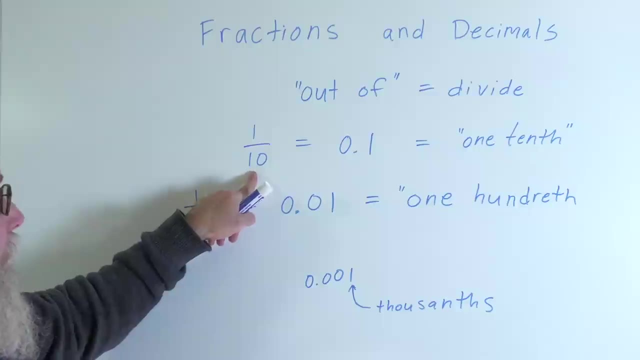 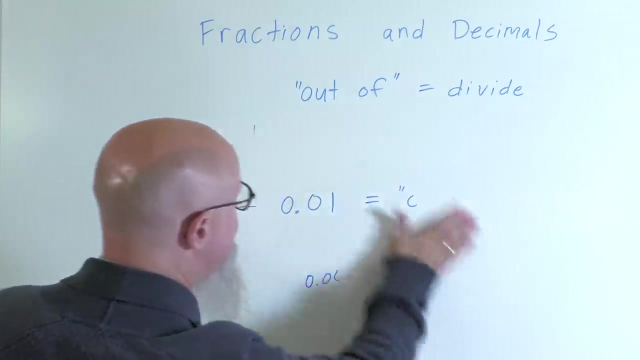 So and it would keep on going. So, knowing that we have that you know tenths, hundredths, thousandths, then that would be our denominator if we want to convert it back the other way. So if I would, if I had something that 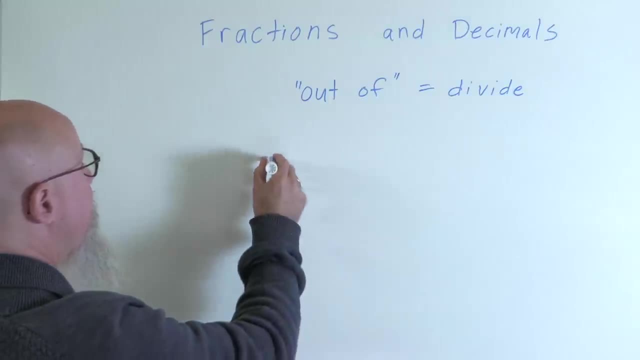 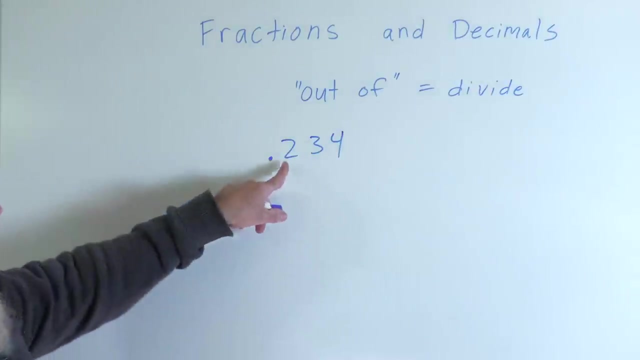 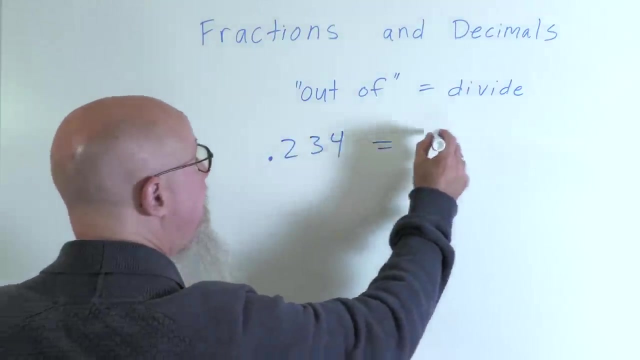 If I would, you know, 0.234,, so something that I wanted to convert- then I would take this as tenths, hundredths, thousandths. that's where it ends. So then I could make that 234 out of a thousand. 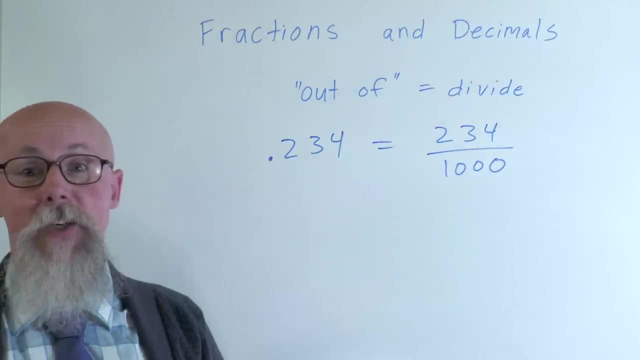 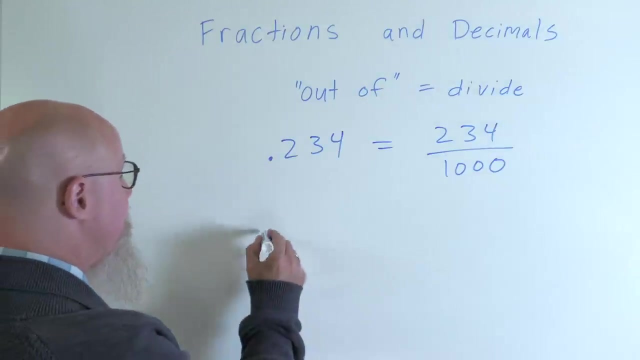 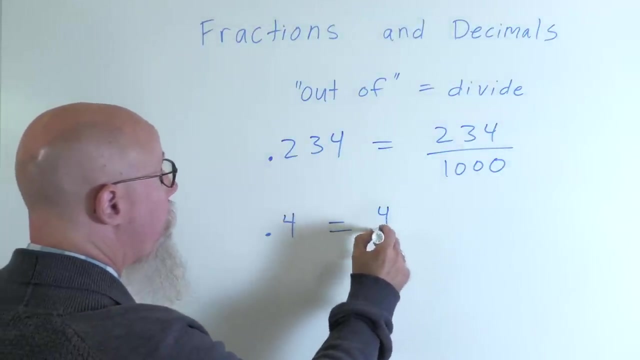 And I could reduce that, but that still is the fraction that I'm looking for. So 234 out of a thousand. Or if I had something you know, like 0.4.. One place that's one tenth, So that would be four out of ten. 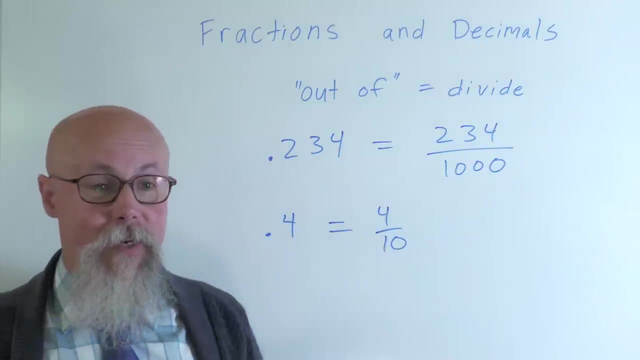 And again I could reduce it or I could leave it as that. You know, that's converting my decimal right to a fraction, And when we get into the code we're going to look at how to See. here I'm just looking at this and remembering these tenths, hundredths, thousandths, etc. 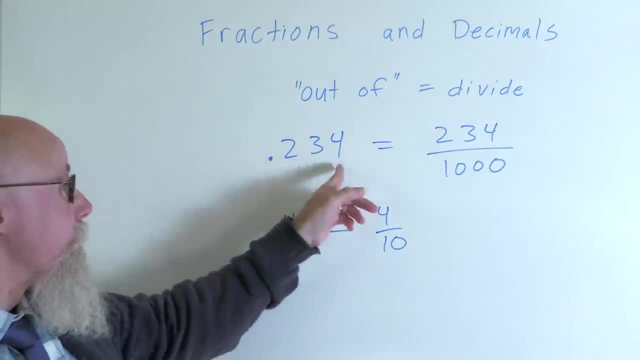 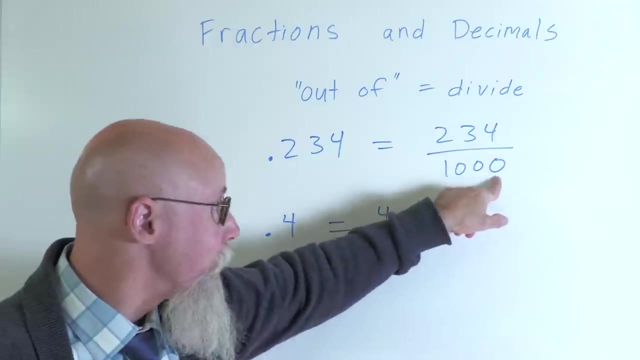 It could keep going. You could convert any decimal, But I'm looking at these, remembering the place values, and then saying: oh, that's three, so I'll have ten, with one followed by three zeros. You know one decimal place, so my denominator is one followed by one zero. 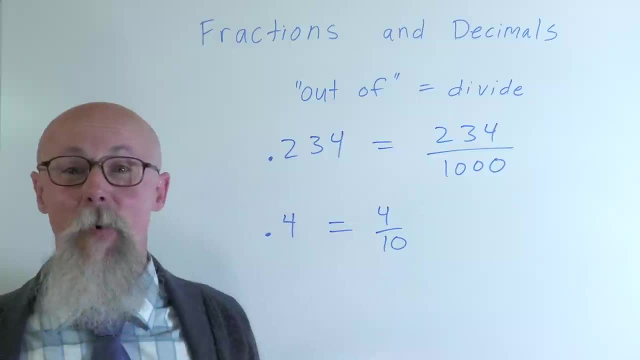 And when we get into the code, we're going to look at how to do that in a different way rather than just: Well, there's a few other ways. you can like take it as a string and count how many places. 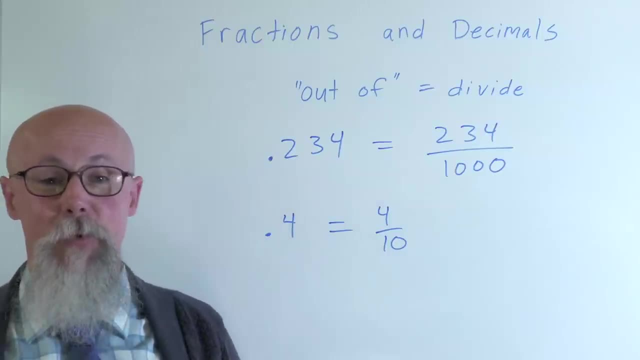 Or you know, one of the lessons we're going to look at: the logarithm, The logarithm way, probably the string and just counting it. that's probably a little more straightforward. We'll do that one, But there we go. 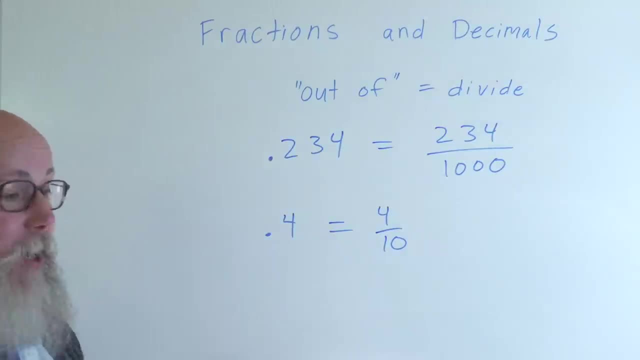 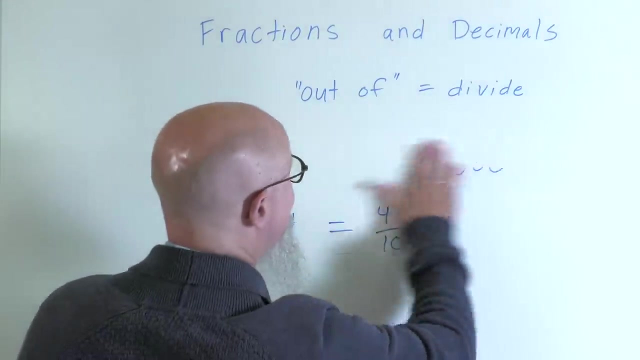 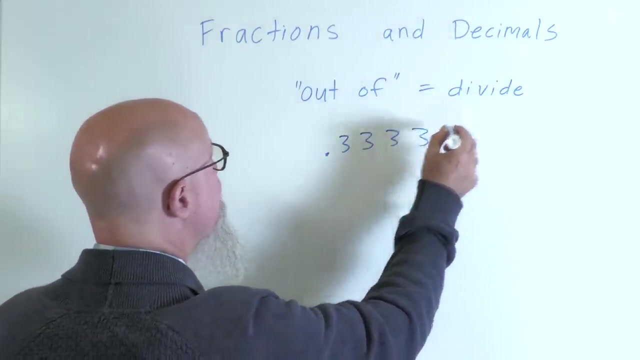 Converting these. you know how do I get this, And then you know how do I reduce it. Okay, so we think we have it all worked out, But what about if I have a repeating decimal? So supposing I have 0.3333, and it keeps repeating? 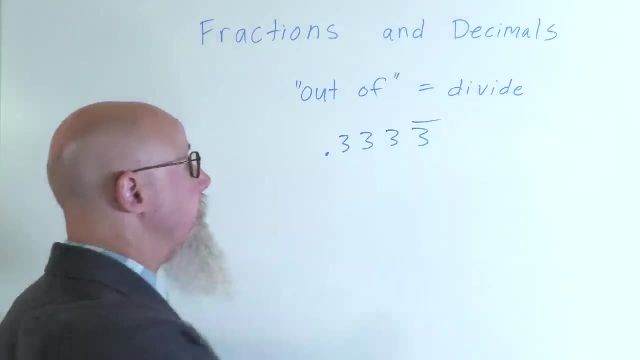 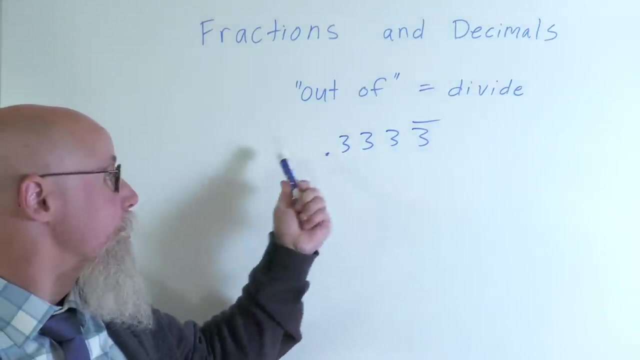 Okay, And mathematically, If I was writing this, you put the line over one of the, the part that repeats, So I really could just keep it as one. but I want to show you three repeats. just put it over the three. 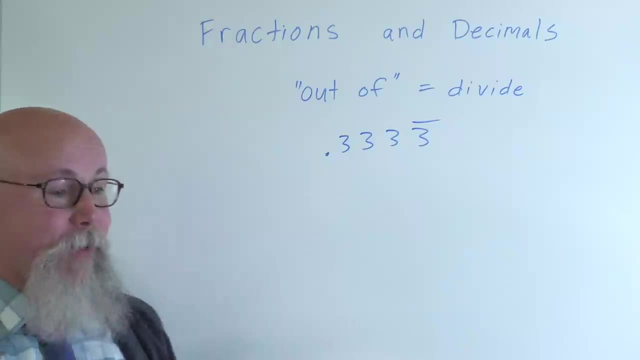 So if that keeps repeating? okay, So we were just talking about you know how many decimal places and then put it over that, But if it keeps repeating, where do I stop? So let's take a look at a trick: how to do this. 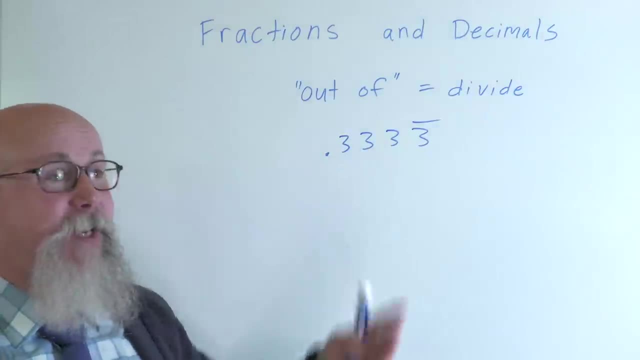 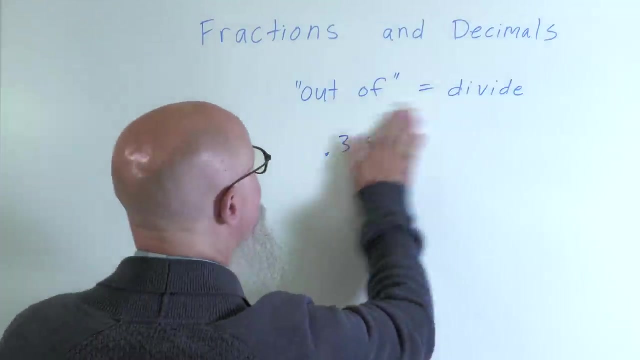 We want to get to the end of the repeating. So if it only repeats once, then If I multiply this, let's let me call this x, And actually I'm going to write this down a little bit further. This is that's going to make sense in a second here. 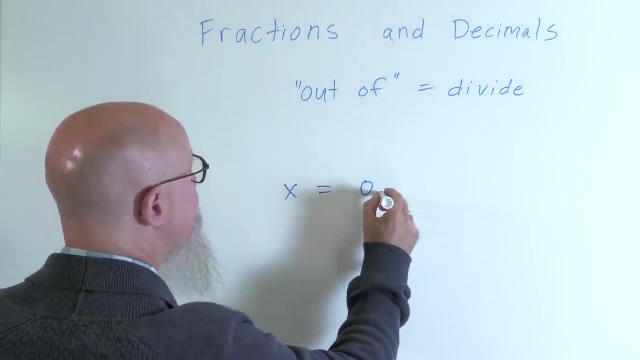 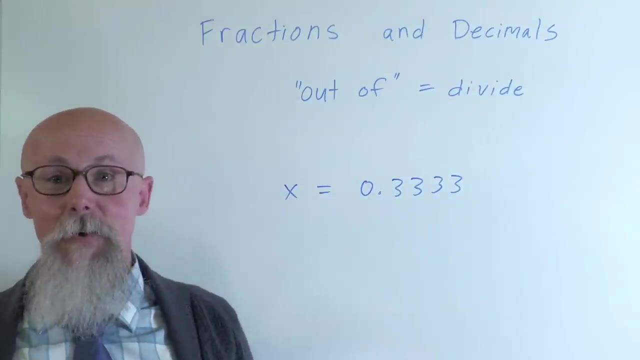 So if I say x is my 0.3333, repeating, All right. So if that's my value, I only need to multiply it by 10 to move the decimal place once, and then that cancels out. So if I have 10x, then that cancels out. 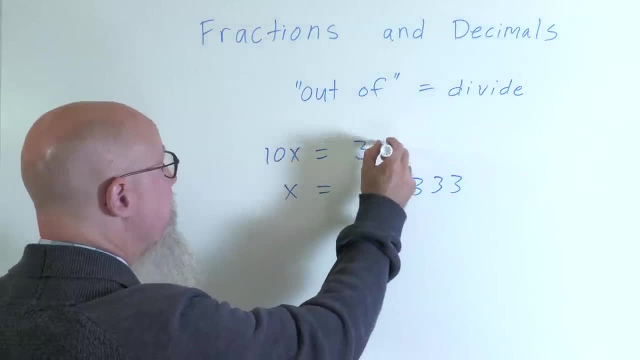 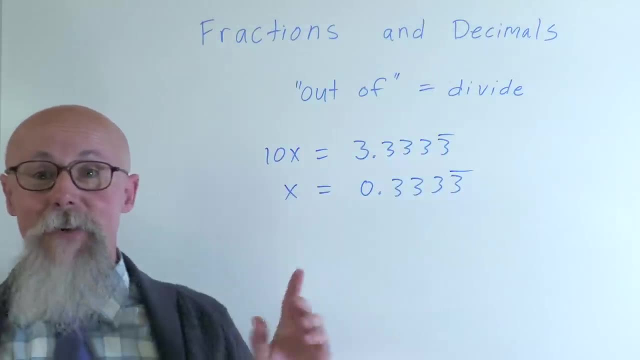 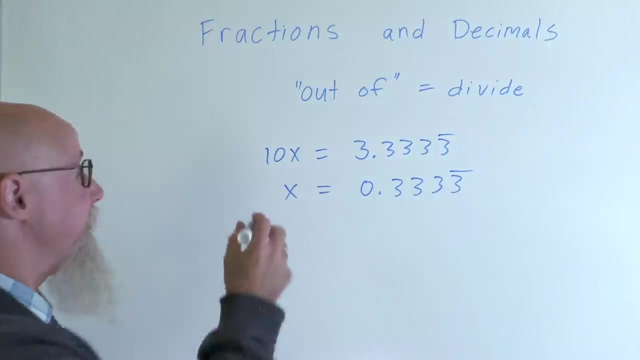 And you know these keep repeating. Now, the reason I do that is because of all the repeating decimals. everything that repeats now is going to line up, And so if I subtract these, what can I do? On the left, 10x minus x is 9x. 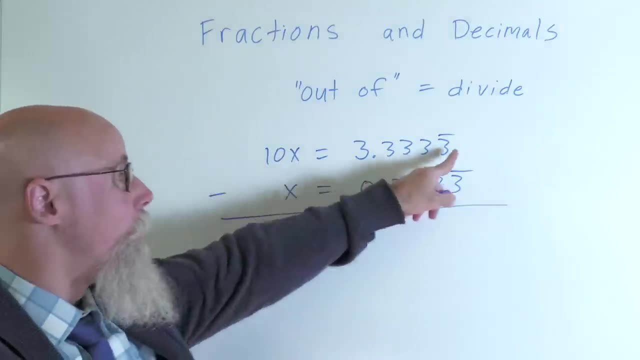 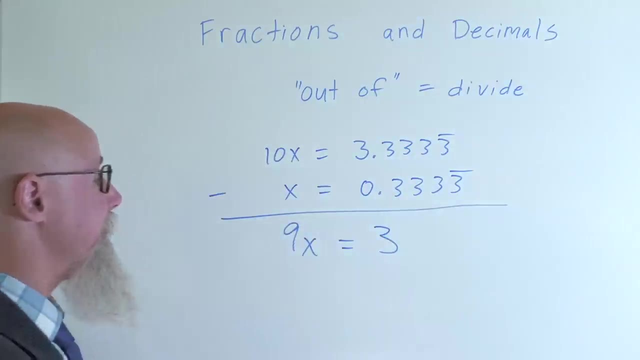 Equal sign is still there And 3.. all this minus 0., all this, That cancels. all this. however many decimal places you want to go, It all cancels and my answer is 3.. And then one step of algebra: solve for x, divide both sides by 9.. 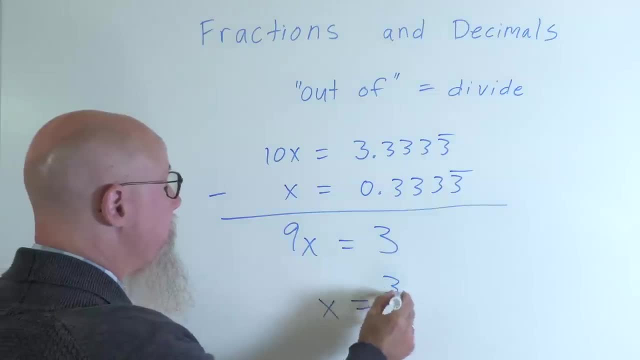 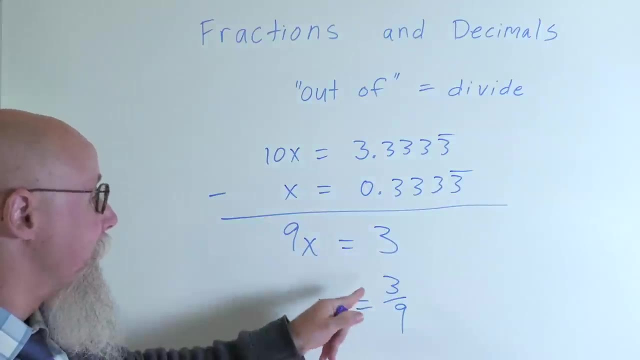 So I get: x equals 3 over 9. Because 9 divided by 9 is 1, so that's 1x 3 divided by 9. And I could reduce that as 1 third if I wanted to. 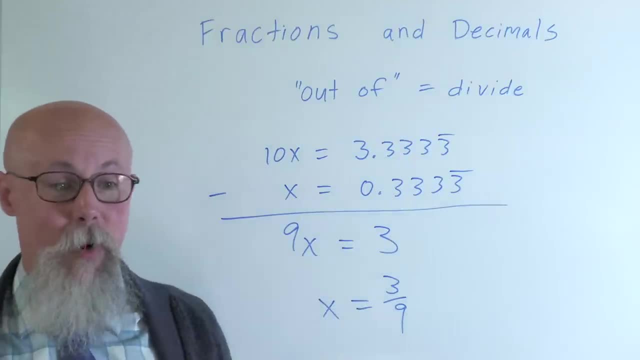 Now keeping it as 3 over 9,. you know, that's nice like bonus Math insight. if I have a single number that repeats, it's that number over 9.. That's the fraction. So if I had 4, if I had, you know, very similar type of question. but if I had something like if I had 0.4 repeating, 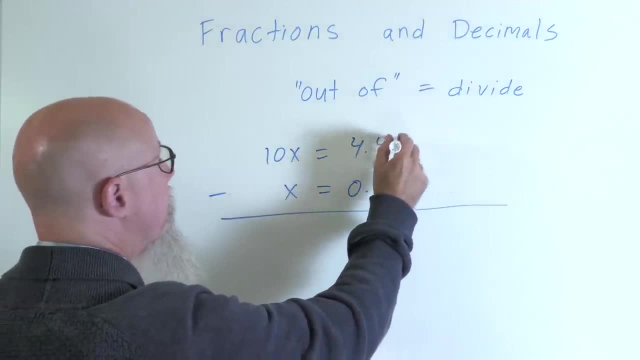 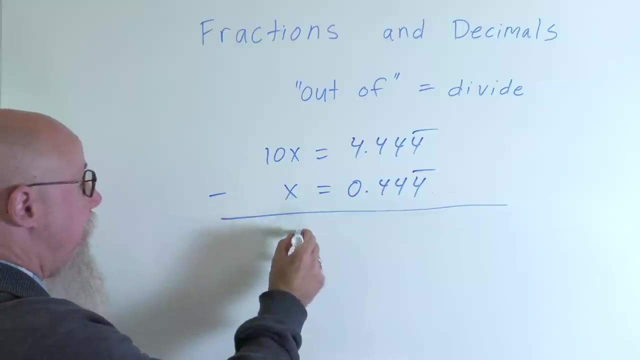 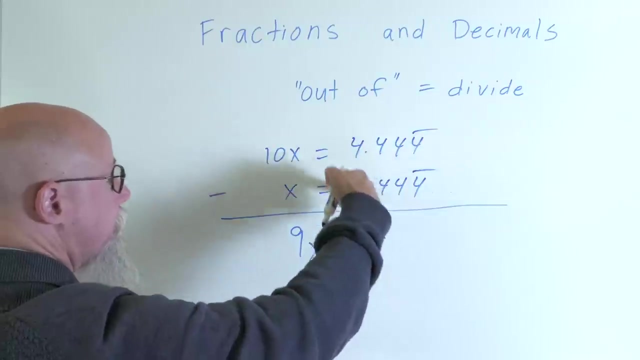 So then 10 times that would be 4.444, etc. They both keep repeating, Do the same subtraction: 10 minus 1 is 9x, And when I subtract these, all the repeating decimals cancel. So 4 point. this minus 0.4 is exactly 4.. 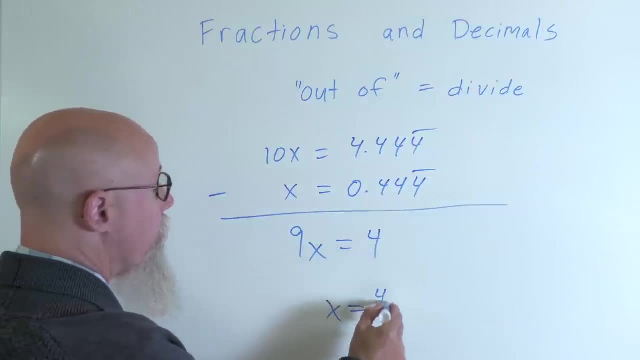 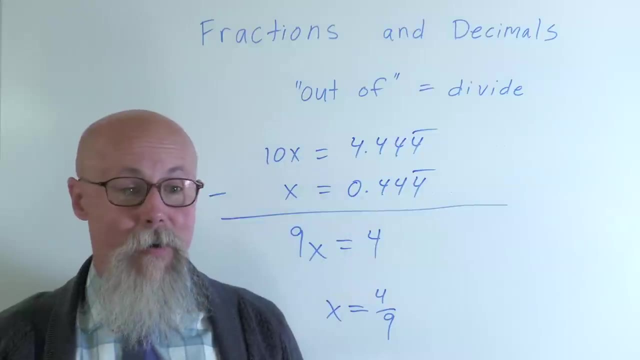 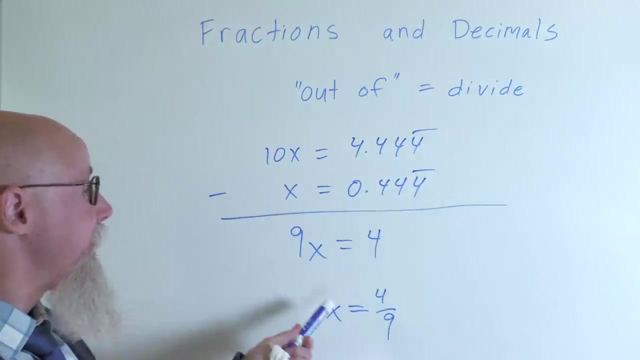 And when I divide both sides by 9, x equals 4 over 9.. So there we go, And so one more bonus here. If I had 9 repeating, we could do the same thing And you would think 0.999, that's not exactly 1.. 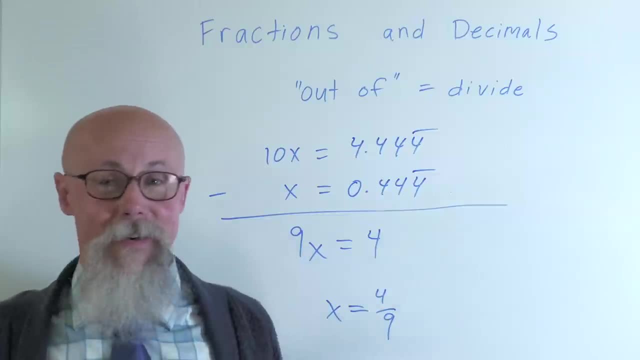 And well, later on in calculus we can look at limits and how 0.9 repeating if it keeps on going. for all practical purposes that is 1.. But if we did this it would be 9s repeating and we divide by 9, and you get x equals 1.. 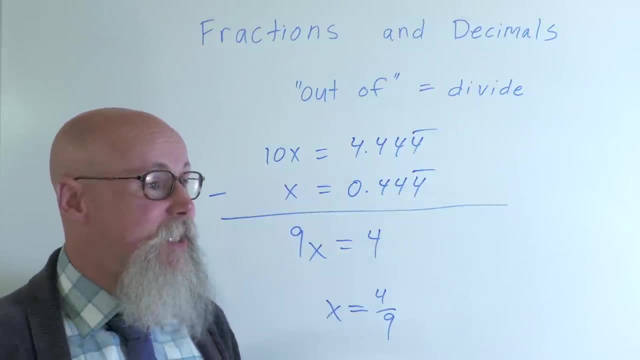 So it kind of works out nicely. But this is how we can do this. You know, notice, we're not looking at code here, We're just taking this, And if we have something that repeats, then that's what we need to do. 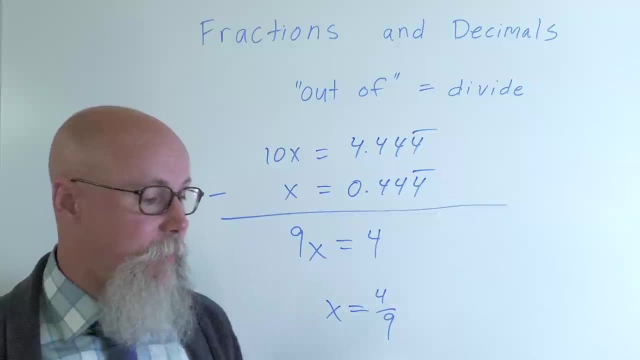 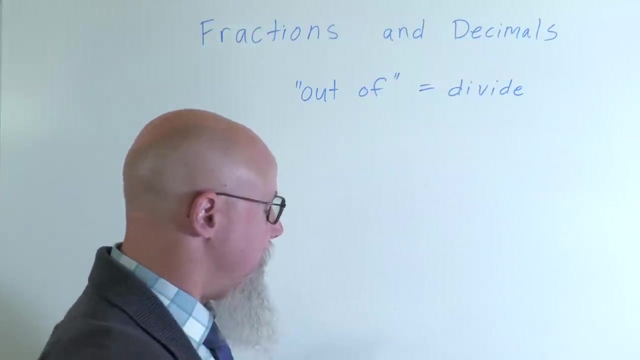 We need to find out where it repeats. If I had something that repeated, you know, two places over and over again. let's do that one. And just to give you an idea of a different way, if I have something that repeats, then if I have so, x equals 0. 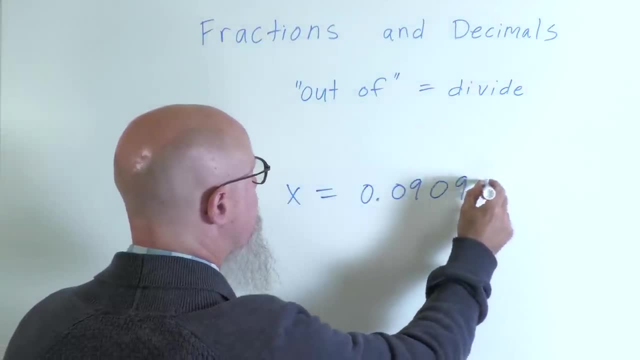 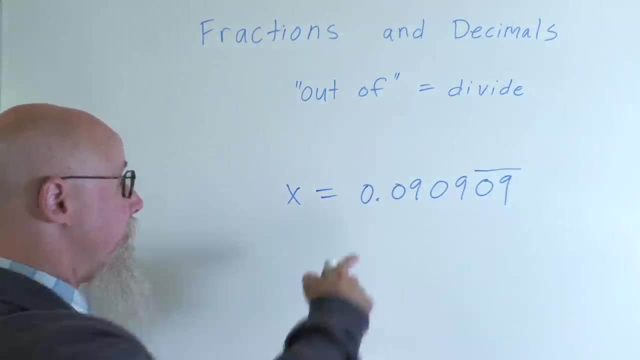 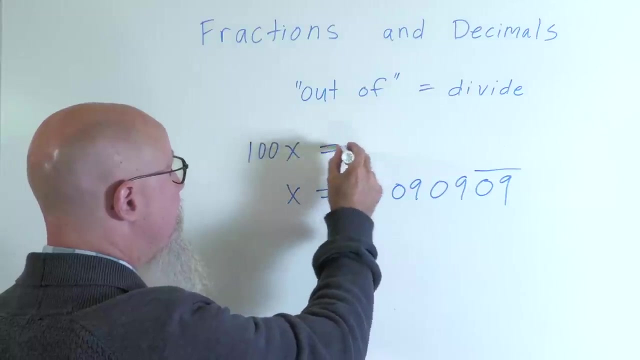 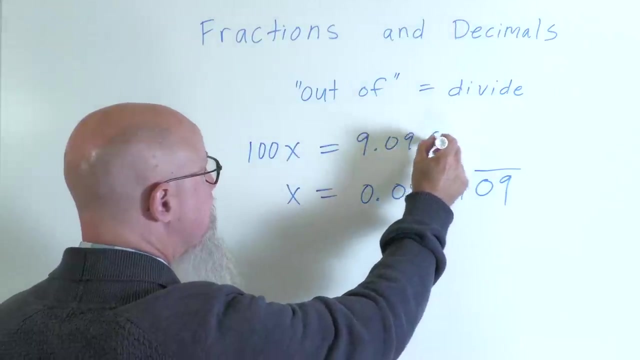 0.090909,, something like that, And it's the 09 that repeats. So I need to multiply it by 100 to line it up So 100x, because that would move the decimal place twice and that makes it 9.090909, etc. 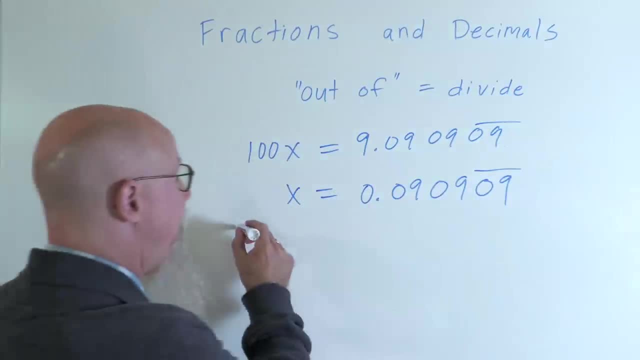 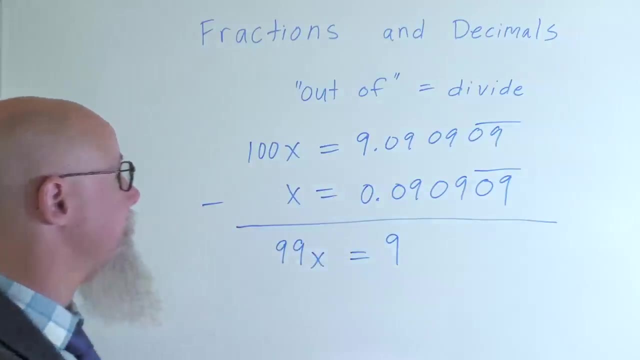 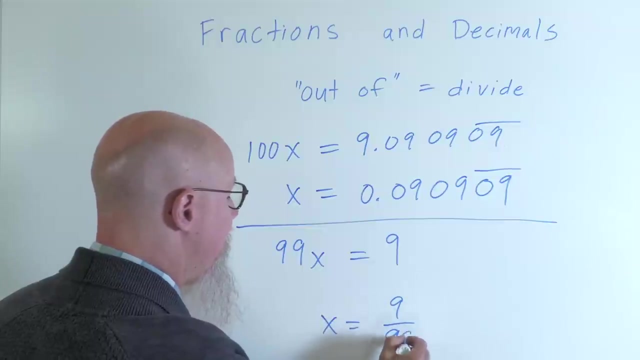 So 1.. When I do that now, same method- if I subtract these, that's 99x equals 9, because the net cancels. So then x equals 99,, 9 over 99. And fine, perfectly acceptable answer. but we can reduce this, so that's 1 out of 11.. 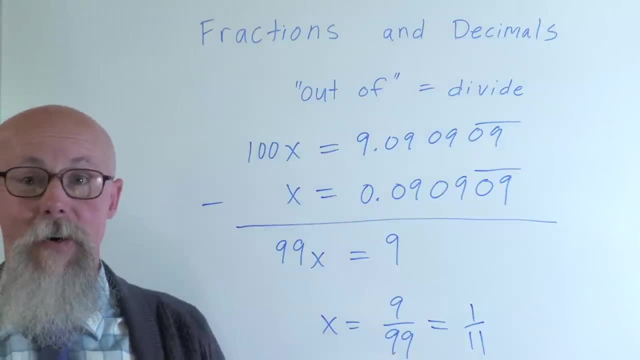 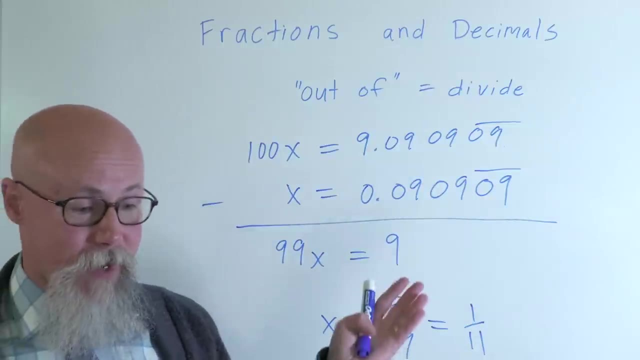 We'll get into reducing fractions and also the code for that too. But you see, this is one way. if you have something that repeats and maybe the way you write the code, it might seem to break it if you don't find some way around it. 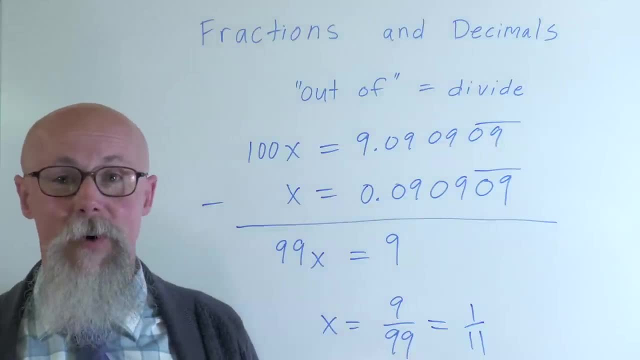 This is the way around it, So we can convert any repeating decimal. But now what we're going to do is we're going to get into the code and how to take any decimal. just here's the decimal input: how can I find a way to count how many spaces that is and reframe that as a fraction? 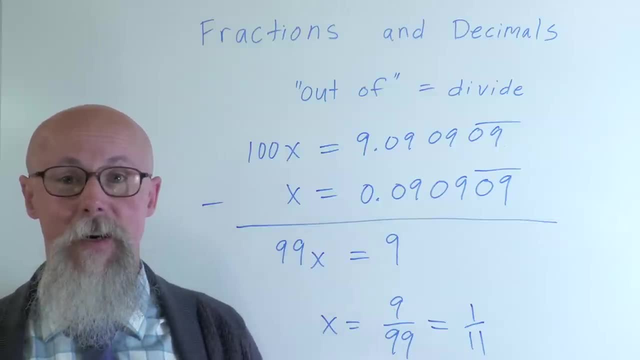 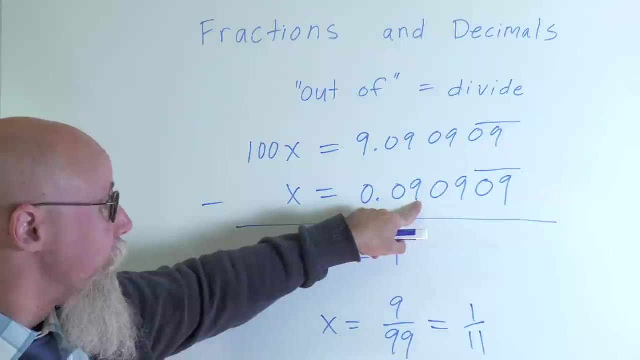 So that, given the decimal, and then we turn it into a fraction, Related to that is percents, because, remember, the first is tenth hundredth, so the first two digits are the hundredths, and that's really what percent means out of a hundred. 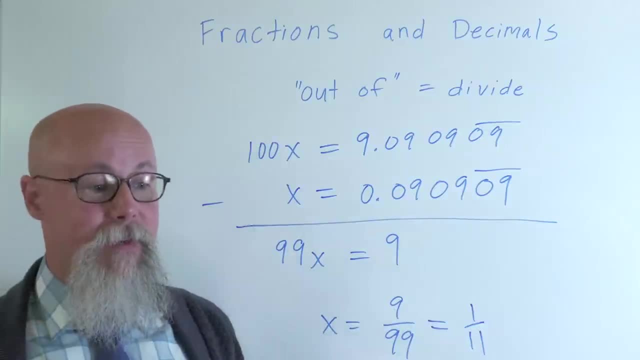 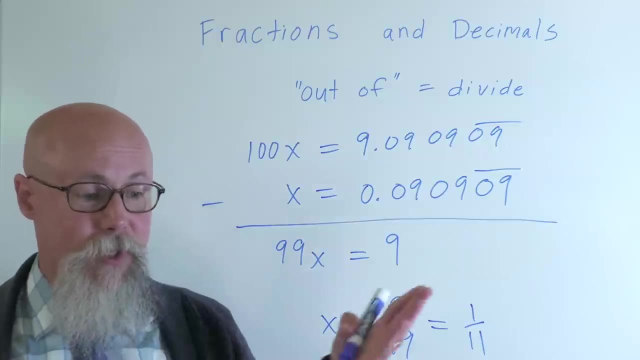 So percent is all the same thing. and then just, I'm always looking at the first two decimal places. that's my percent. So you know, very similar, but just the first two decimal places. So let's take a look at the code and we'll see how it works. 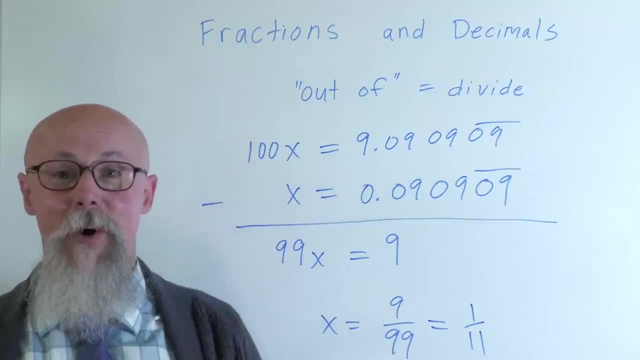 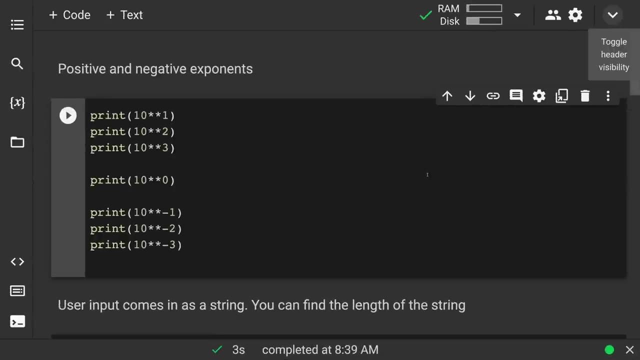 And then we'll see how to convert any decimal to a fraction. Alright, So let's talk about how to convert decimals to fractions with code, And first we'll get some background here, because this is going to be useful. 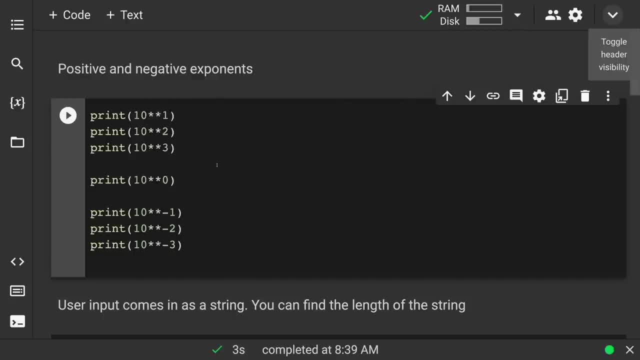 So if I have ten, two different exponents, let's take a look at the positive exponents. So ten to the first power. we see this first one. ten to the first power, ten to the second, ten to the third. 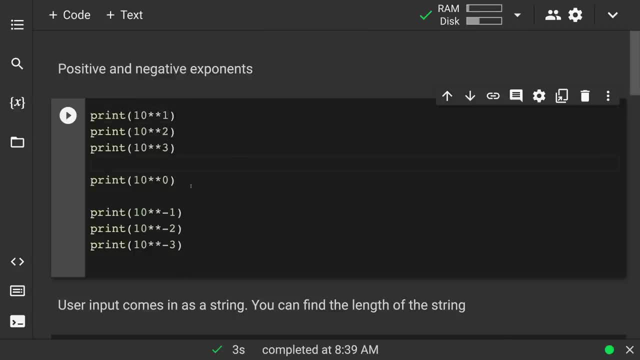 We'll see these come up. what happens when we take ten to a positive exponent, Ten or anything else to the zero exponent, And then we'll take a look at ten to the negative one or negative two or negative three. So this will just print these out, but let's take a look at what this does. 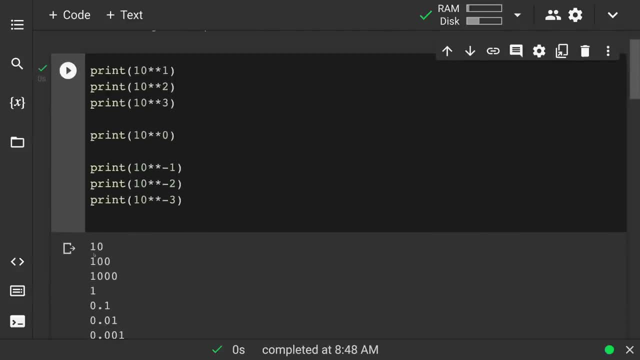 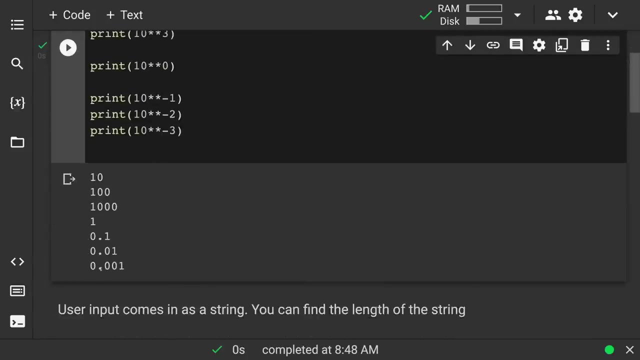 So we see, ten to the first, second or third becomes ten, a hundred, a thousand, Ten or anything to the zero is one. And then the negative exponents are: how many decimal places Point? one point, oh one point, oh oh one. 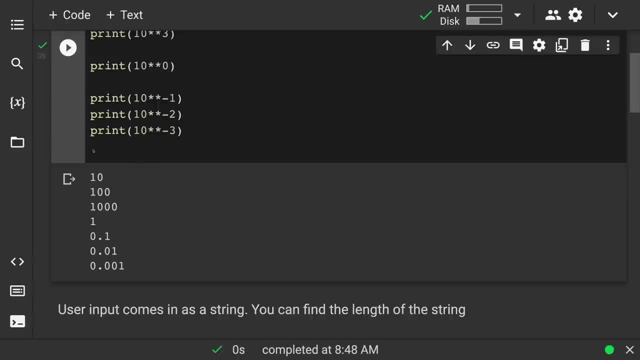 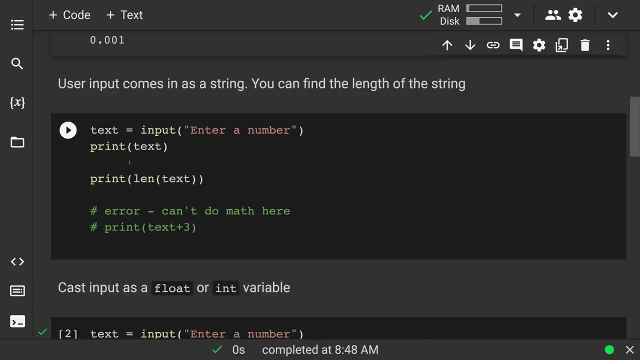 So these are the things we're looking for and we're going to make use of this as we convert our decimals to fractions. So the next thing: we'll take a look at how to get user input And we have this formula. 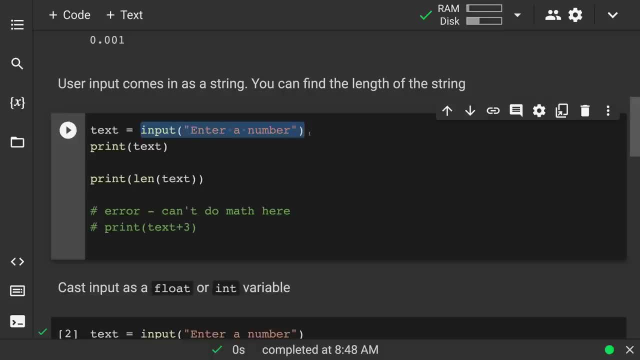 Here user input, open parentheses And in quotes here this is what it will display, And then you'll see then a box, you know, then asking for input, And then here we're going to store that as text, as that's the variable. 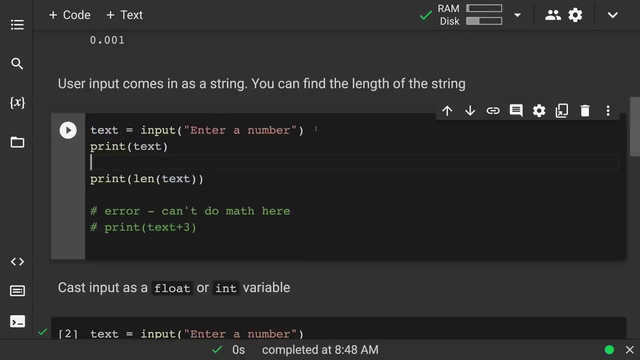 For our purposes here. we're just going to show you that you can enter a number and we're going to print it out. I call the variable text, just to remind you. it comes in as a string. We can't do any math with it yet. 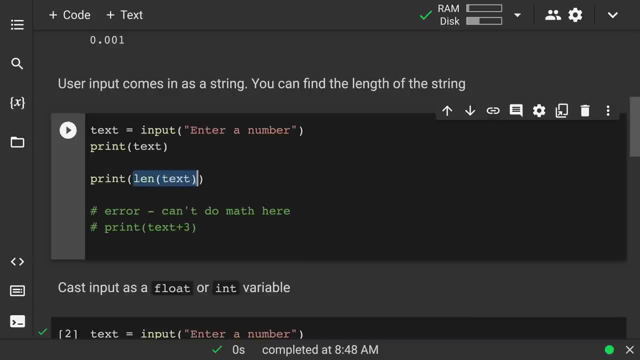 But one of the things I can do: any string, I can figure out the length of that string. So we're just going to print that out. And I just have again this comment here. if I tried to do math with it then there would be an error. 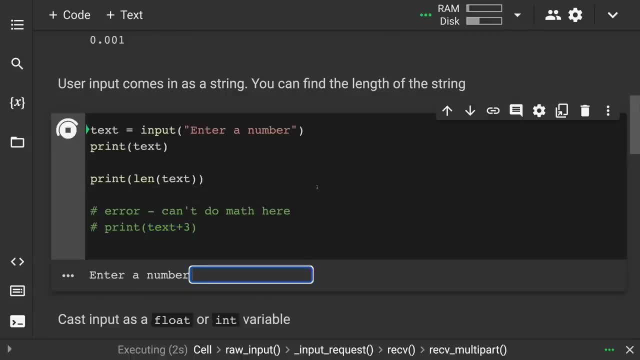 So let's take a look. So you see enter a number. And then if I had a number with a decimal like point one, two, three, I hit enter. You see point one, two, three. 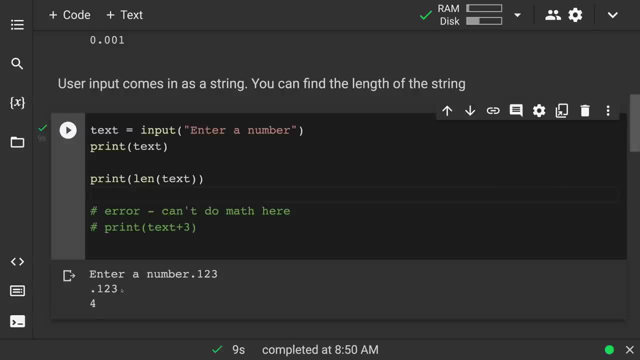 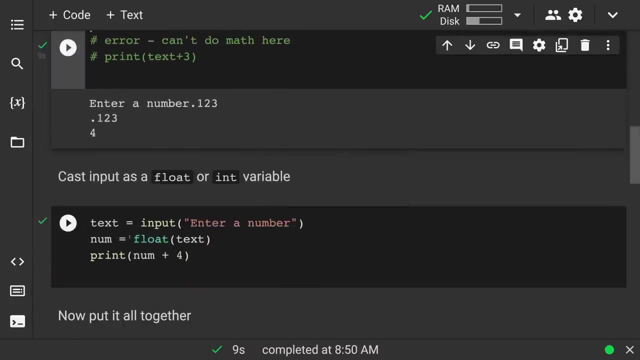 The length of it is four because there's a string. These are four characters. The decimal point counts as one character. So different things I can do with this. So you know, if I wanted to enter a number now, if I have, if I cast it as a float. 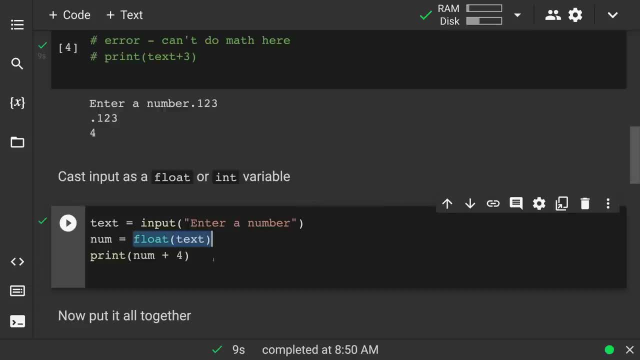 now I can do math to it And I can cast it as a float or an int for integer. So just keeping in mind, you know things I might want to do with this. A float can have decimal places, So that's usually my default cast. 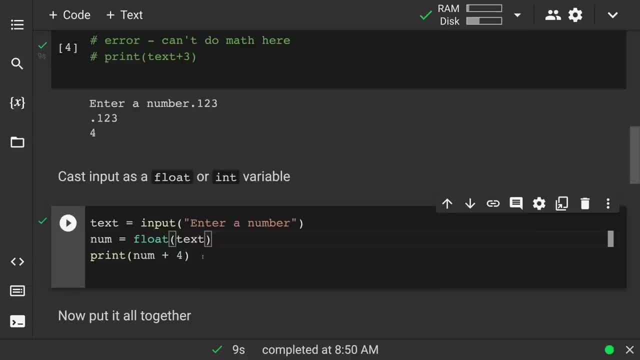 But you know, if you definitely know that you want it to be an integer, we would use that. But we're going to enter a number, cast it as a float and store it as the variable number num. Now I can do math to it. 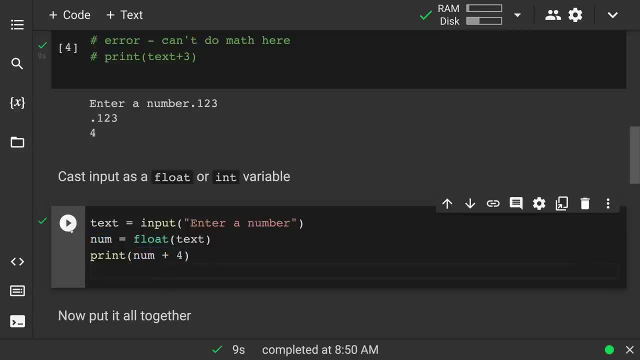 I'm going to print out num plus four, So we'll see, There we go. If I enter a number, there we go. And if I have point one, two, three, then hit enter. You see, now I can. now I can add. 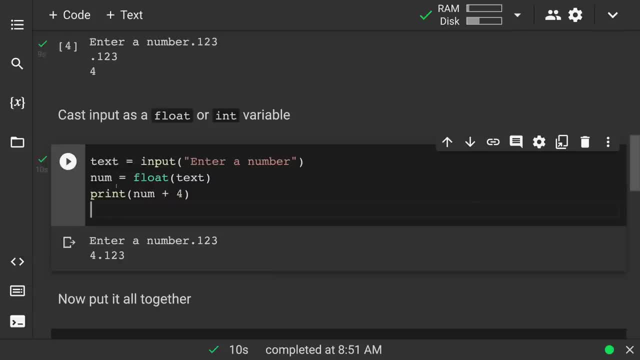 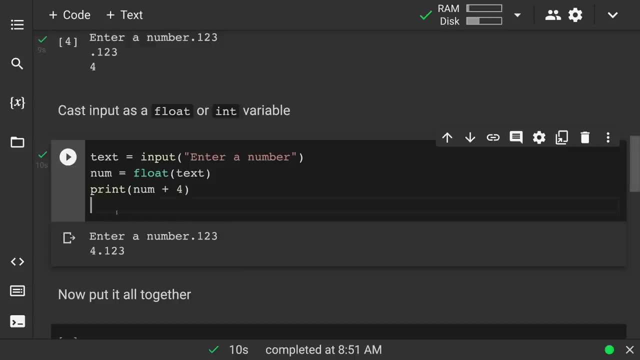 Alright, Or whatever other math operation you want. Once you cast it as a float or an int, then you can do math to it. And the float because it can handle decimal- any math operation that there might be a chance of a decimal. 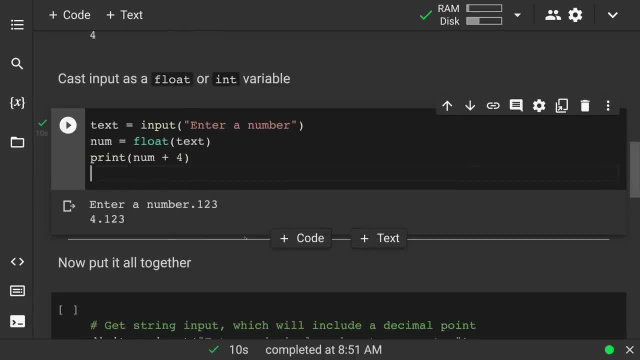 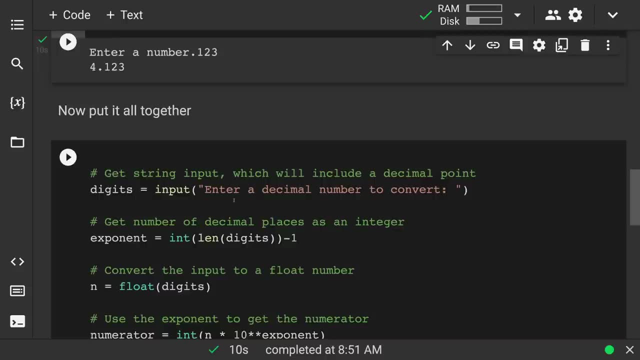 use float. Okay, So we're going to put all this together, So converting this input, which will come in as a decimal. So I'm going to take this input and here's what I'm going to print out. 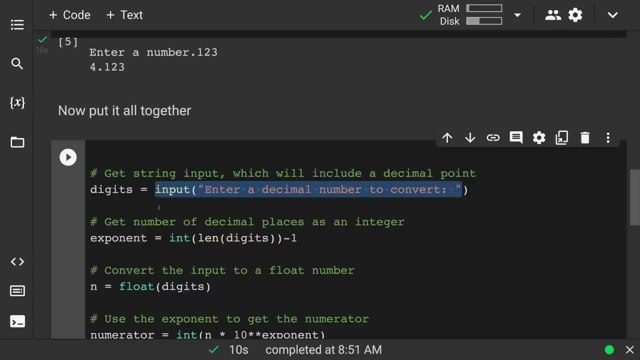 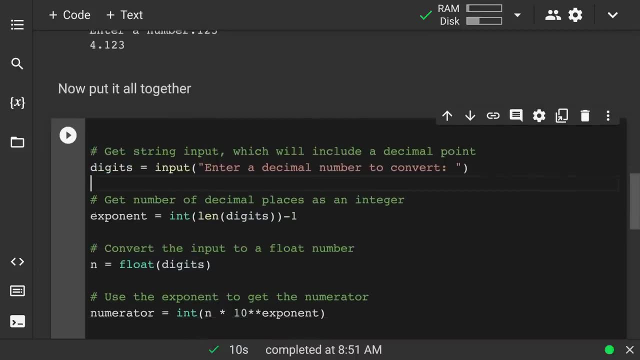 Enter a decimal number to convert. There we go. So we know that that's input and that's going to be stored as digits and we know that that's going to be a string. So to get the number of decimal places, 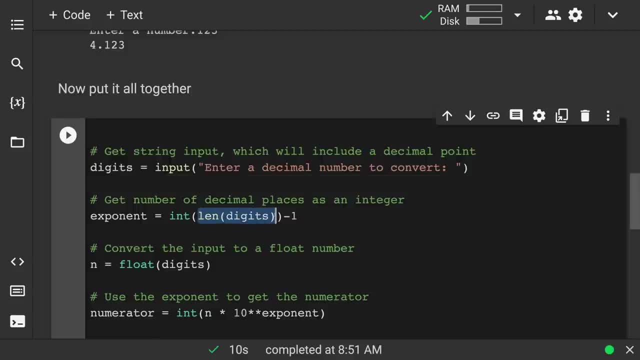 the next thing. So I'm going to use this: Notice the length of that input digits And I'm going to cast it as an integer first. So notice that happens first. Then I'm going to subtract one. 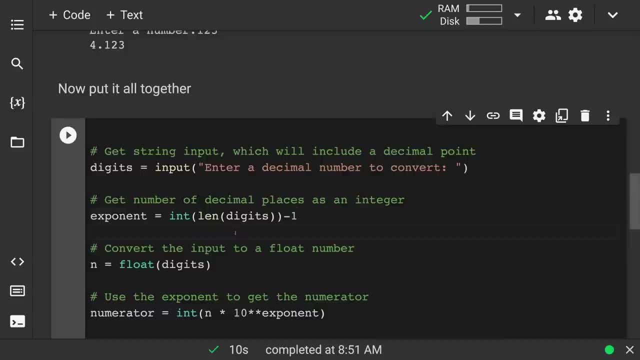 Because, remember, as a string, that decimal point's going to count when I do the length of that string. So I want to subtract one because I don't want that decimal. So now, whatever decimal enter minus the decimal point itself. 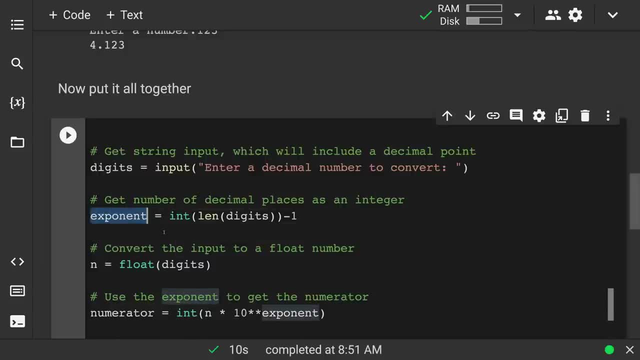 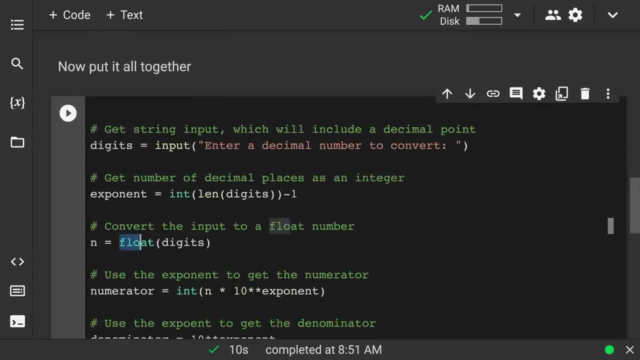 that's going to be an integer, that's going to be the exponent. And now here I go back to digits. that is still a string. Now I'm going to cast that exactly as a float number. I'll store that as n. 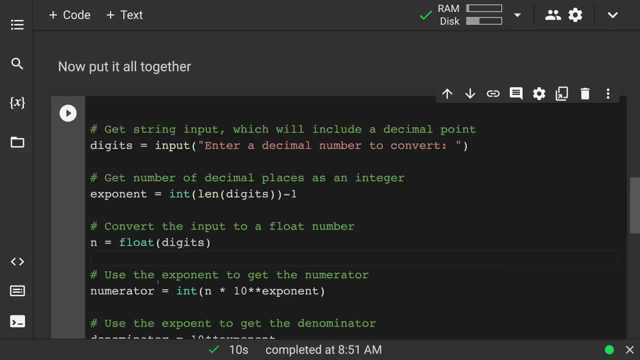 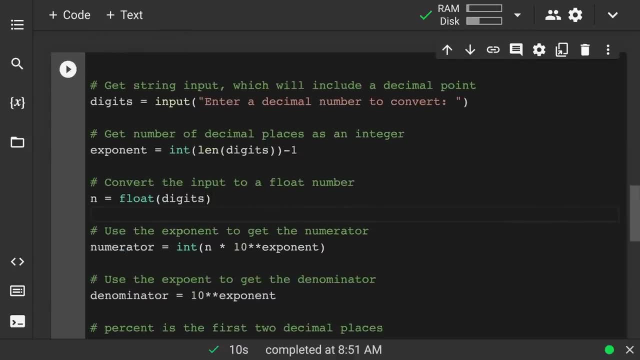 So now I know how many decimal places it took to make that, and the number itself is a float. So let's talk about our fraction. My numerator is going to be n times 10 to a certain exponent. 10 to that exponent. 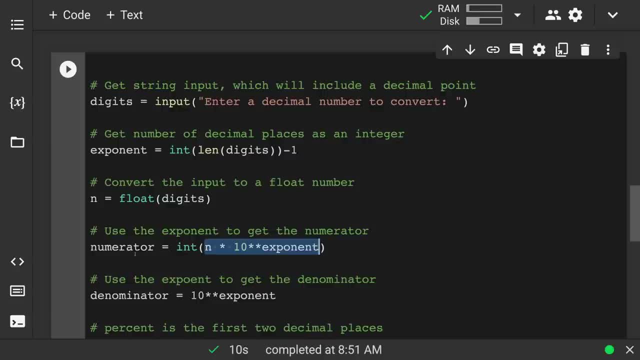 So in my previous example 0.123, then it's going to be. you know that was 4, the length of that was 4, so minus 1.. So the 1,, 2, 3. 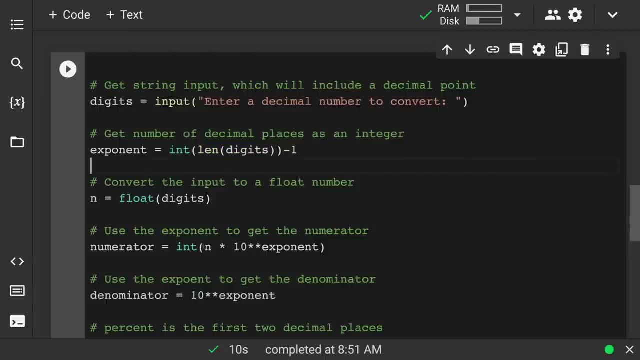 becomes my exponent, And then when I multiply it by that exponent, it makes it a whole number, And since I know it's going to be a whole number, I will cast it as an integer. So that's going to be my numerator. 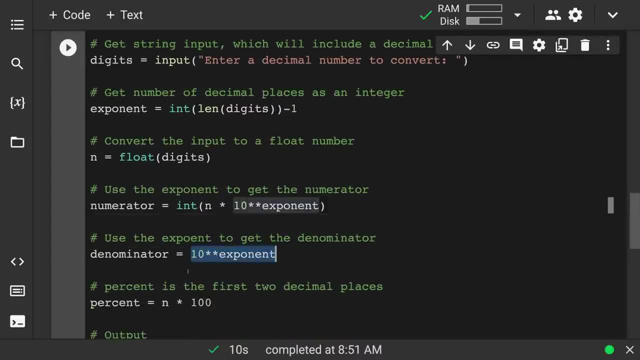 And then the denominator is going to be 10 times that exponent. So you see, that is what we were doing before. we were doing the code. You know how many digits, how many decimal places, and then you know. 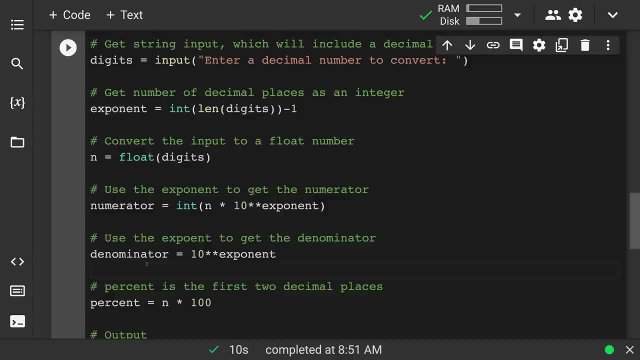 my numerator is that times 10 to that exponent, just 10 to that exponent, So three decimal places would be that times 10 to the third, and then the numerator and denominator would be 10 to the third And it gets you that decimal place. 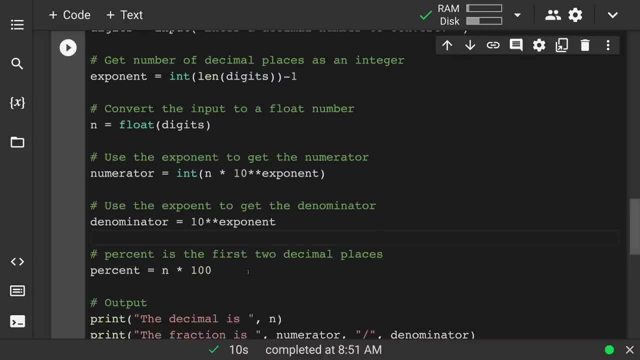 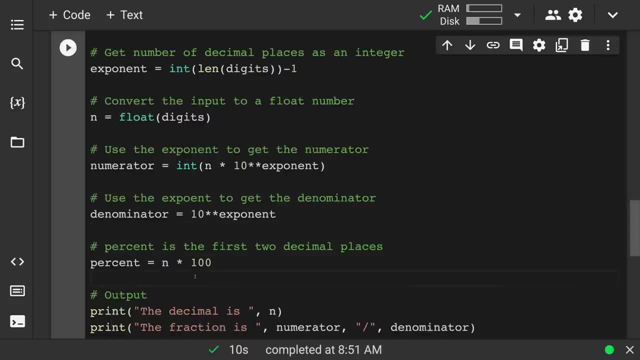 Now that's numerator and denominator for any fraction. Percent is just the first two decimal places. So whatever n is, I'm going to multiply it by 100. Because then that just gets the percent, That decimal move, the decimal place twice. 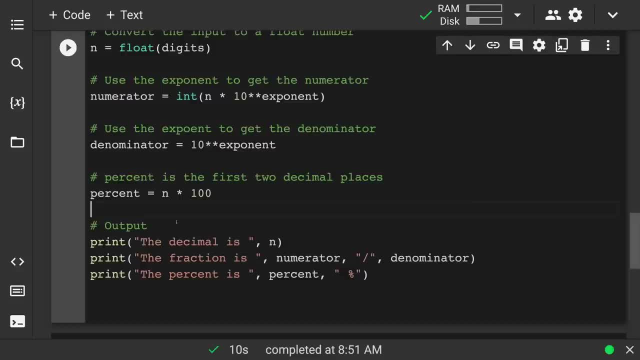 which is multiplying by 100.. So now we'll see the output, the decimal. There we go. We just repeat the decimal again, The fraction numerator, and I'm just going to print this out to show you it's: numerator over denominator. 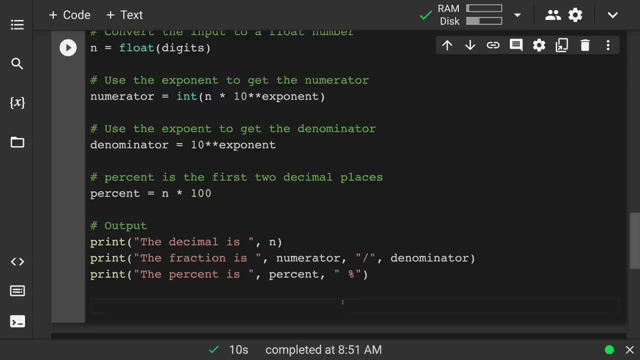 and then the percent, And then I'll print out the percent symbol. There we go. This, remember, in math means something else, but here I'm putting it in quotes, so it'll just be the percent symbol. So we're going to enter a decimal number to convert. 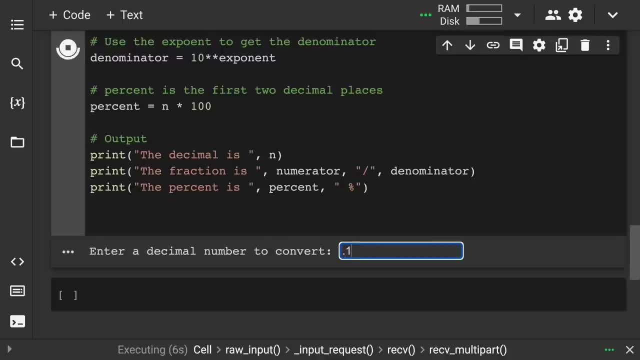 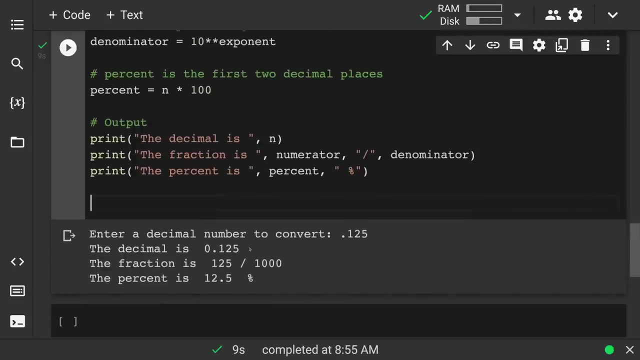 And there we go: 0.125. Enter, There we go, The decimal 0.125 And then the fraction is 125 out of 1000.. That's correct, And the percent is 12.5.. And we can run this again and do this for. 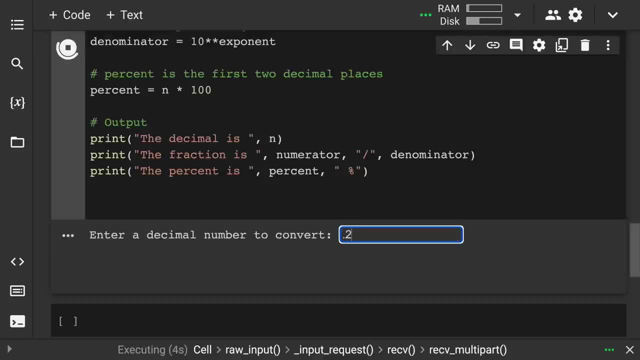 however many decimals we want, You know 0.2. Enter, So it's 0.2, 2 out of 10, or 20%, And there we go, The same things we were doing, And this is what we want to look at. 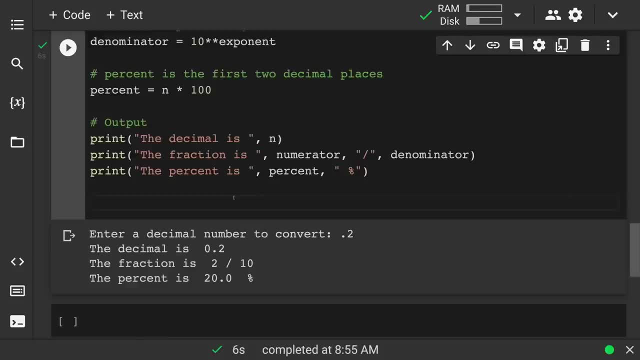 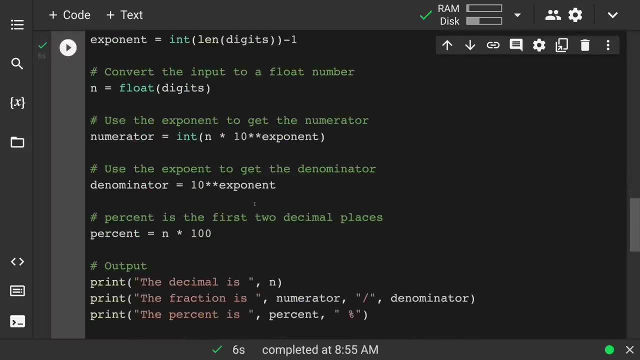 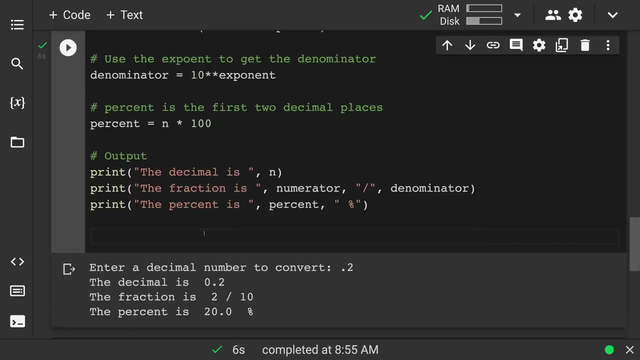 throughout this course. You know the steps that we're doing. in math. we can break this down and we're pretty much doing the same steps. but then now, once we have this written in code, then you know you have a formula that you can reuse. 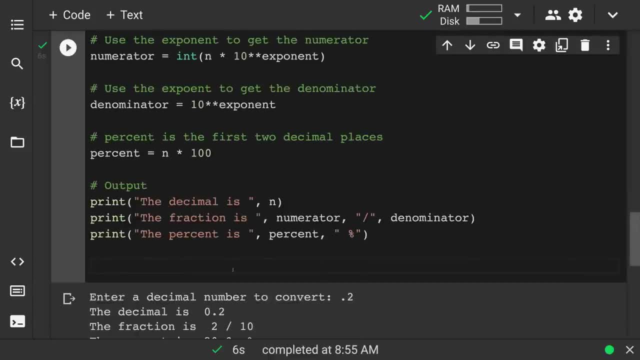 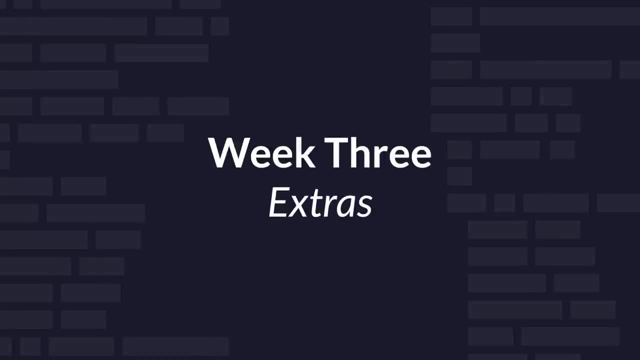 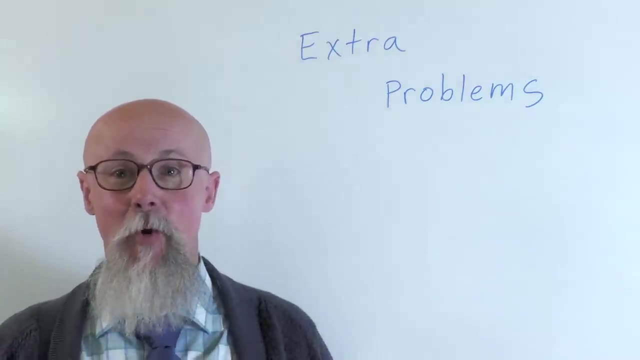 Okay, I'll bring up this script here and I'll be able to convert any decimal to a fraction. There we go. Now that we've worked through the core skills in this unit, let's look through some extra problems, and I'm going to work through. 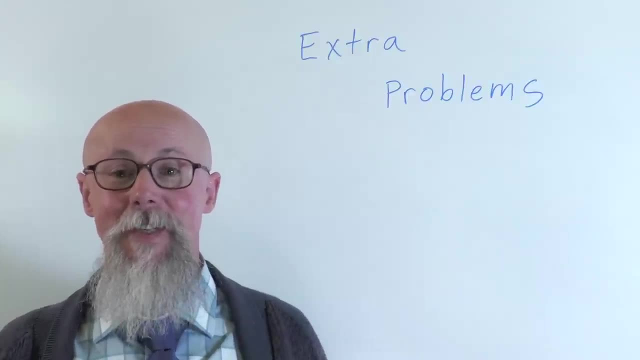 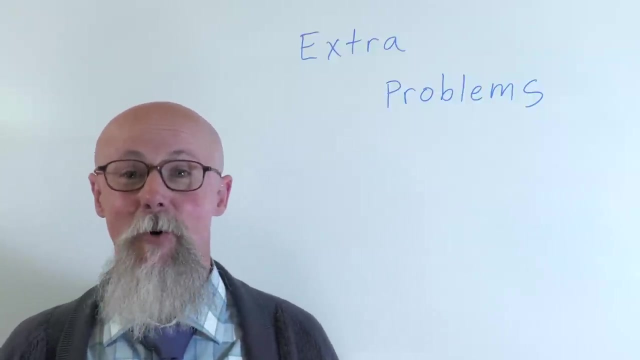 extra problems using the Colab Notebook, So you can see how you can apply these resources that you're building and use these to solve problems that might come up in a textbook or in day-to-day life. So we're going to go through. 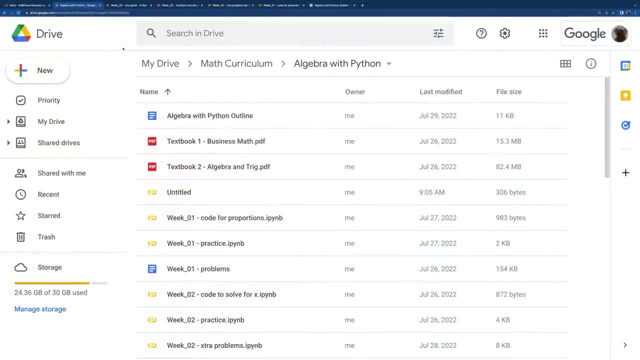 some more extra problems here. So now I want to show you how to put together your own calculator. You know this is what we're talking about here. You're making resources for yourself. So in all the things that I'm showing you and you'll have. 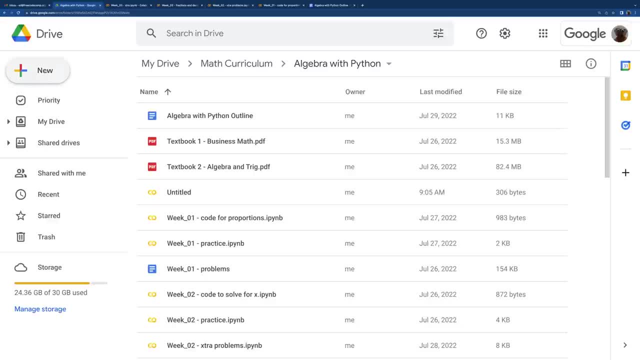 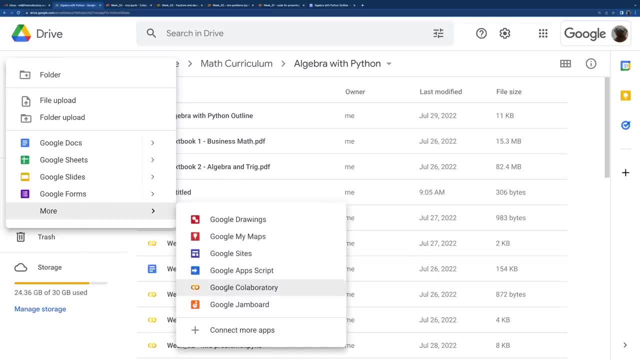 access to all these different resources here, but you're going to put together yours, So you're going to click on New and you would have already added the Google Colab. So go over to Google Colaboratory, click on it. 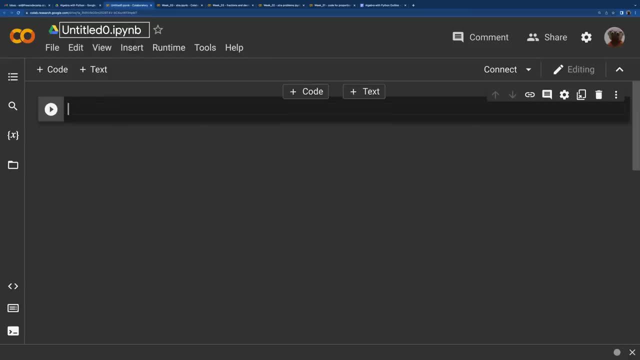 and now this is going to be yours, So actually I will call it that. I'm going to put the underscore. It accepts spaces though Your calculator And you can just hit Enter or click somewhere else, and there we go. So 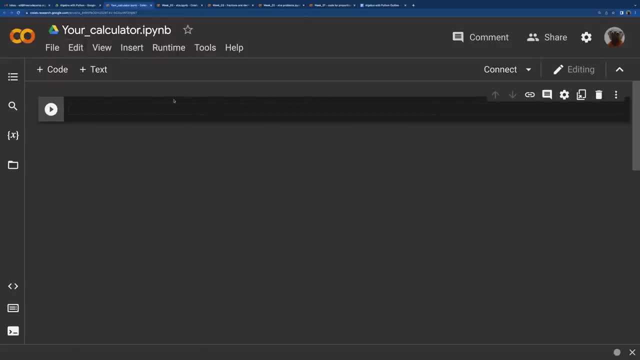 this is what you can do: to put together your calculator based on things that we've been doing so far and then things that we do further on in the class. Then you can add to it, So you can go through and go to, let's say, 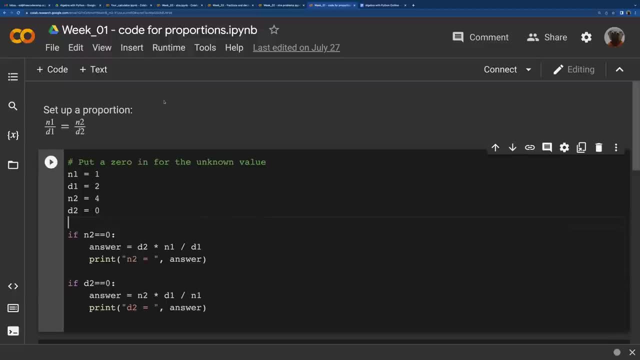 the Week 1 Notebook where you solve for proportions And here's some things you can do. So if you click on this text here to set up the proportion, let's copy that first. So you click on that text and 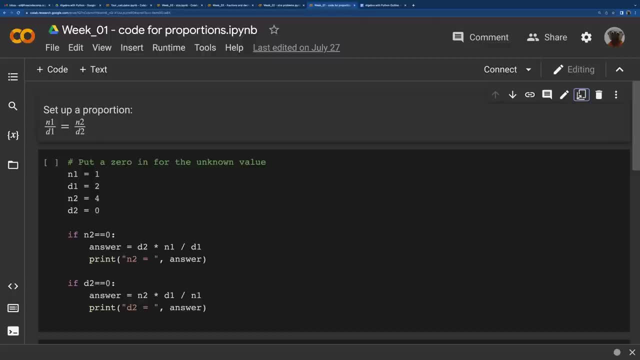 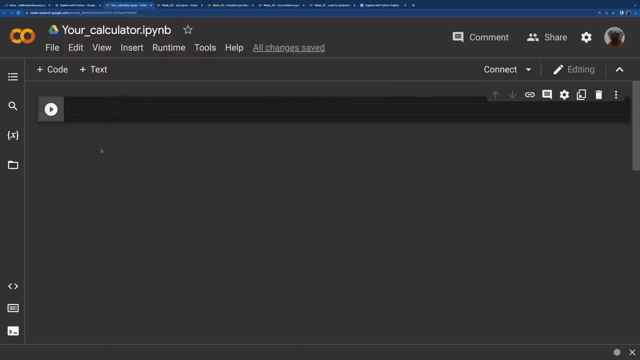 go all the way over the three dots. This looks like copy, but it actually doesn't do what you're expecting it to do- Click on the three dots, copy that cell and when you go back to your calculator- I'm just going to click in the open space here- 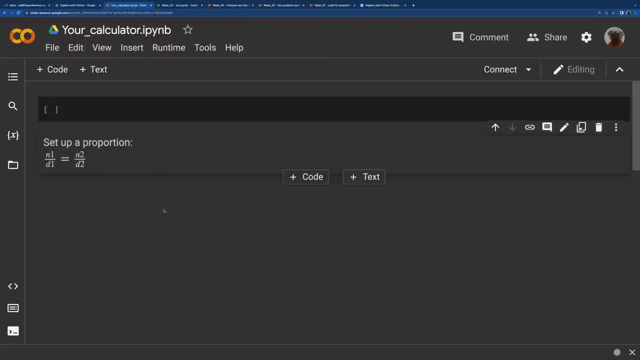 and paste it, Control-V or Command-V- Actually it's kind of cool. So you know, Control-V for the Windows, Command-V for Mac, and Colab accepts either one And then we can go back. That's your proportion. 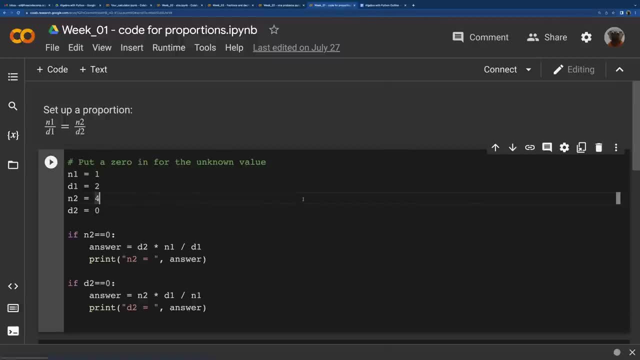 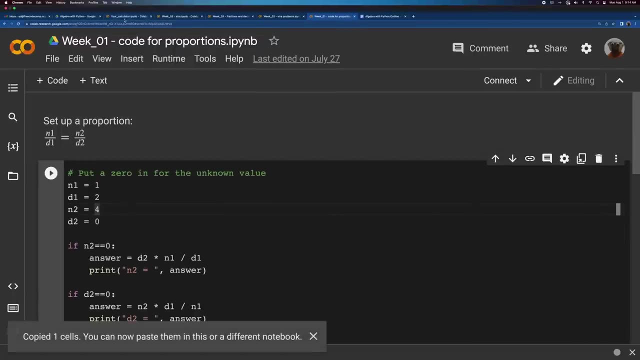 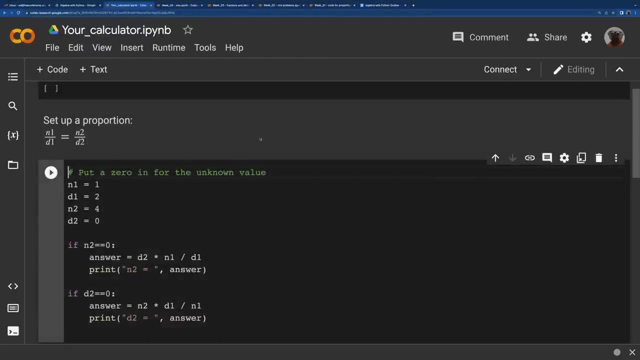 set up there And let's copy this Again all the way over the three dots, copy cell and your calculator and we're going to paste it So you can have this. you know we don't need this If you have an extra one. 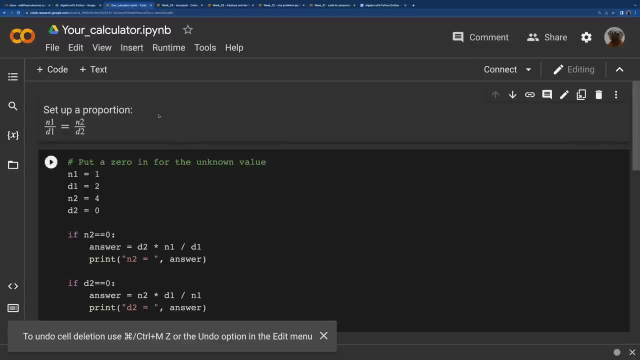 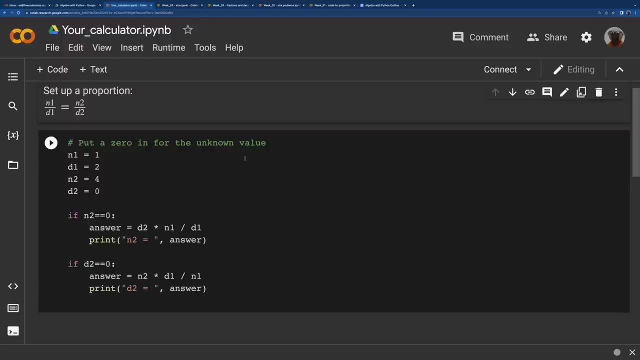 that one, the trash can over there. So there we go. Now you have your text set up, proportion, and then it really is then self-explanatory. You know, you see the set up and put in N1, D1,, N2, D2,. 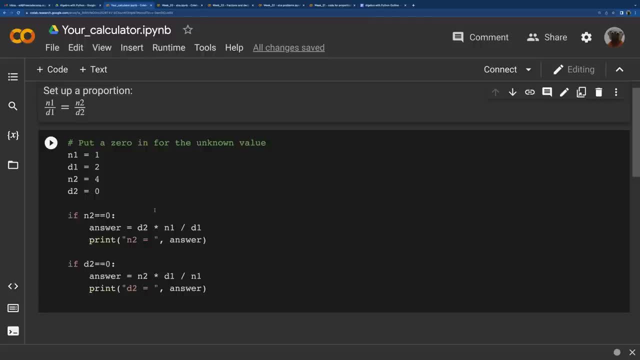 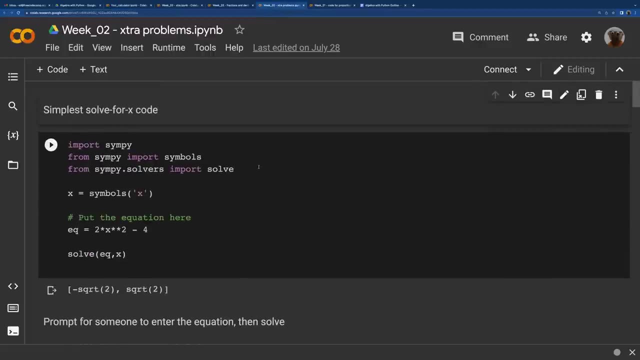 and even the comment there put the zero in for the unknown value, So you can go through each of these. Then, if we look at week two, now we were doing a lot of things for solving for X and maybe you don't need to do. 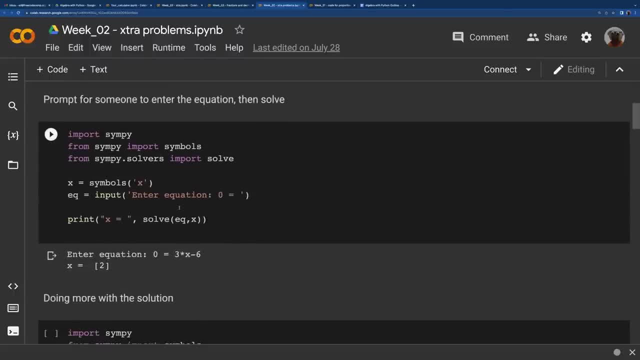 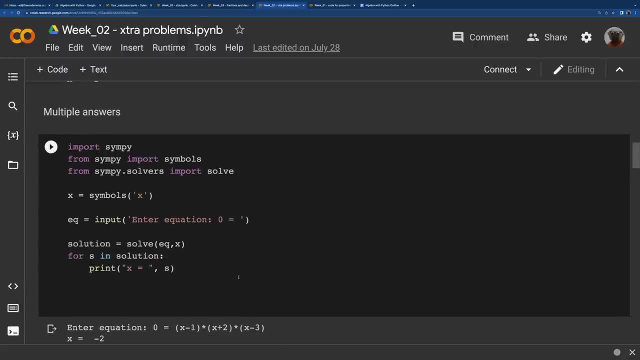 the simplest one. Maybe you like the prompting. You can include that Doing more with the solution, how we split it up Now I personally I like this one, so that might be the one that I copy as one of them, and 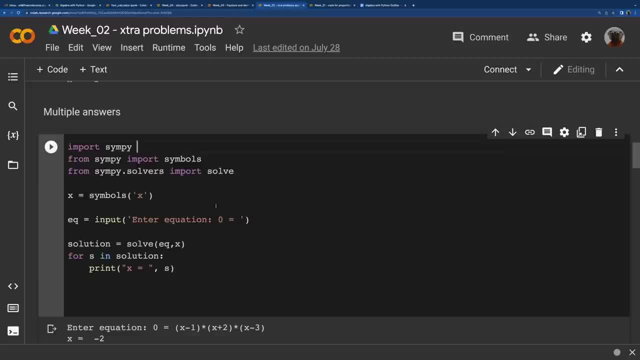 what you can do is, you know, click on here, because notice this one. it I personally like this one. It prompts for the input, already showing that it's something equal to zero. You know, there we go. We already have X as the symbol. 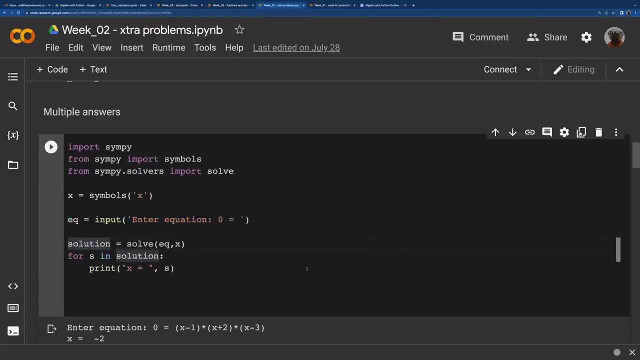 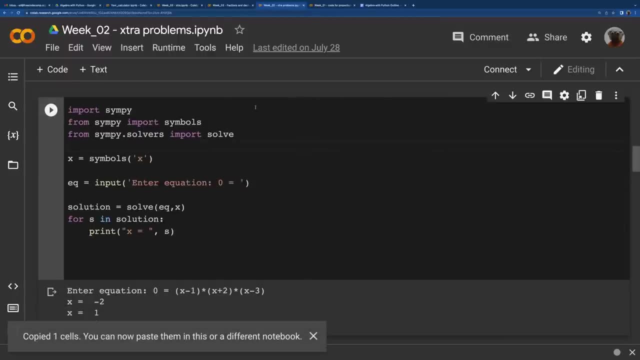 and then this also prints out multiple solutions, if you have them. So this is nice, We can copy this. and when you go back into yours now, if I just paste this, that's great. I actually don't need that. 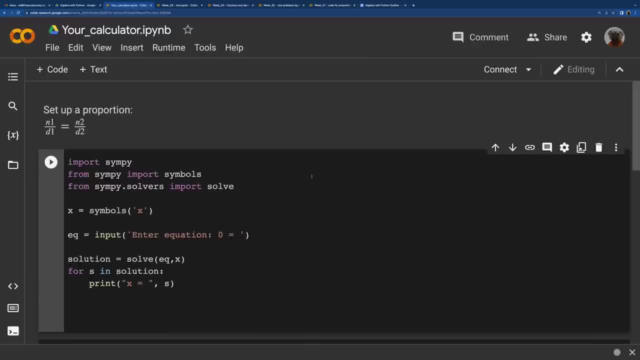 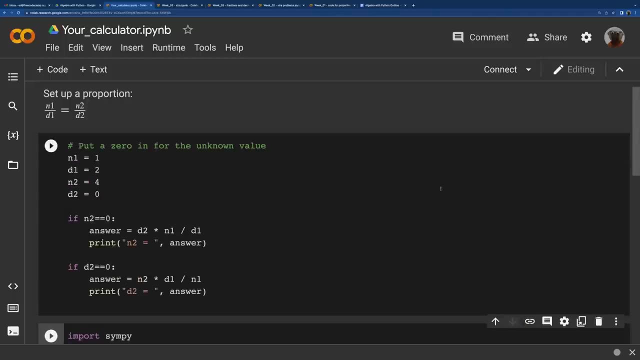 and notice it didn't paste where I wanted it to be, so watch what we can do here. I'm going to click in here and use these arrows, I'm going to move it down and actually down. one is just fine Now. we wanted 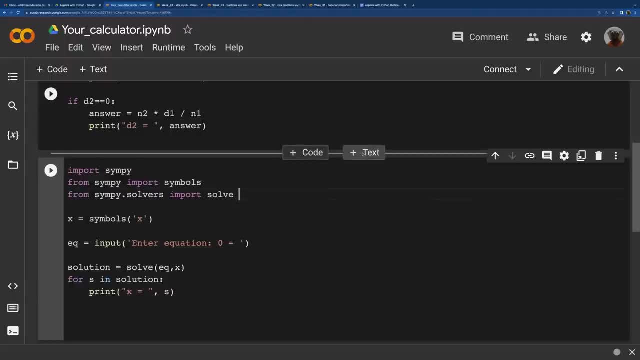 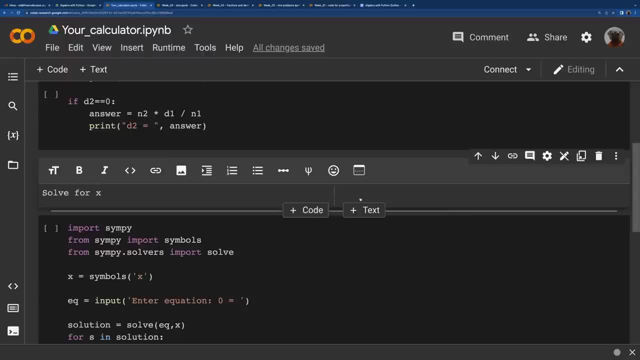 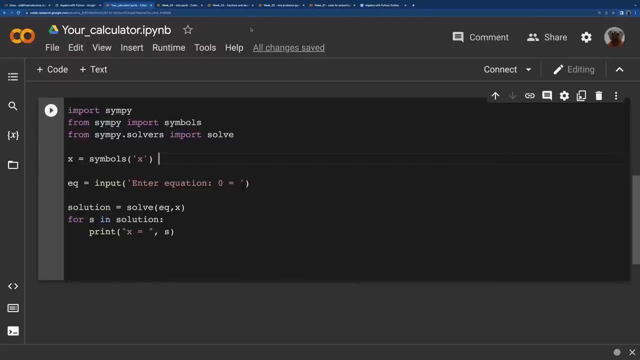 some text in there. so right above it you hover there, add text and solve for X. Maybe I'll just add that text there. So there's more from that week. So we have that. that's nice. Now this solve in other ways. 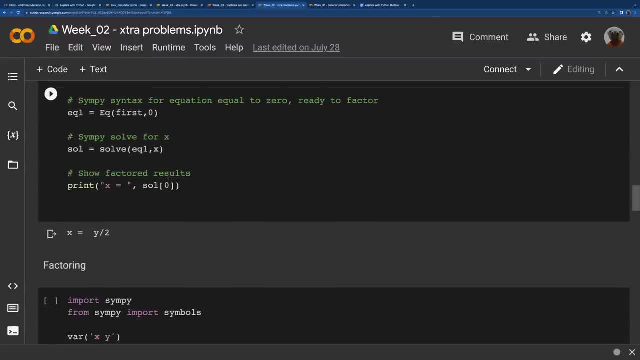 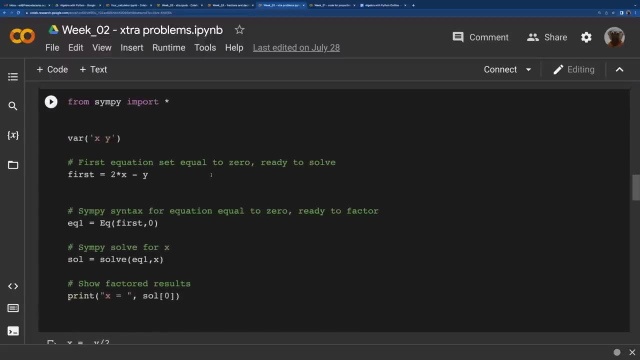 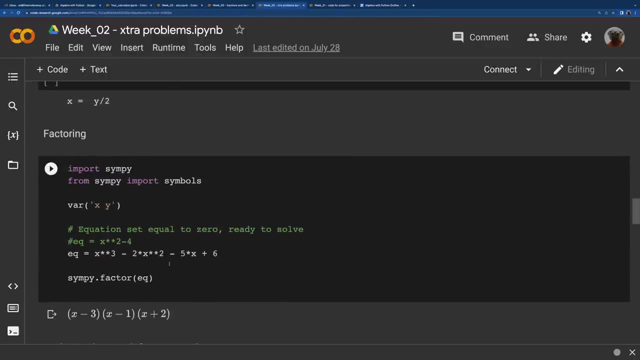 that was pretty good. And then notice there's also factoring, So you could include something like this: solve in other ways or factor, You know, sympyfactor. Now I might include this because you'll see, we'll come back to. 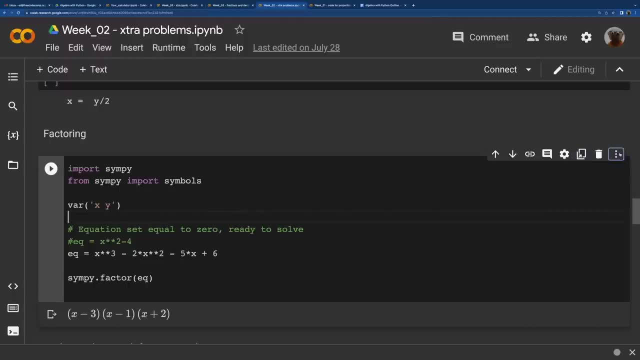 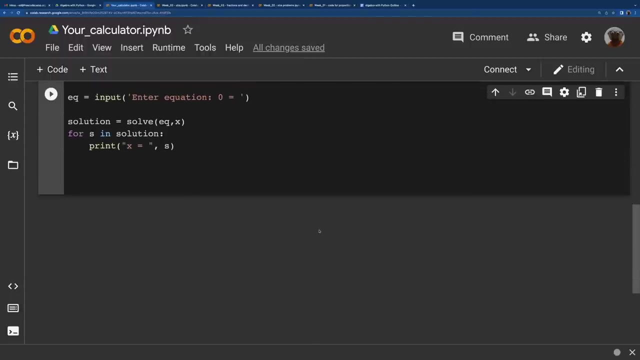 one of the other ones. So if we copy this- and this is just factor, when there's nothing else to solve, You see, So maybe we'll copy this cell and paste this down here Now, maybe I'm going to add text and just put: 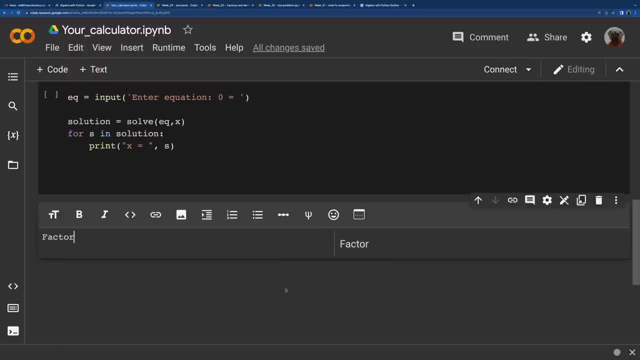 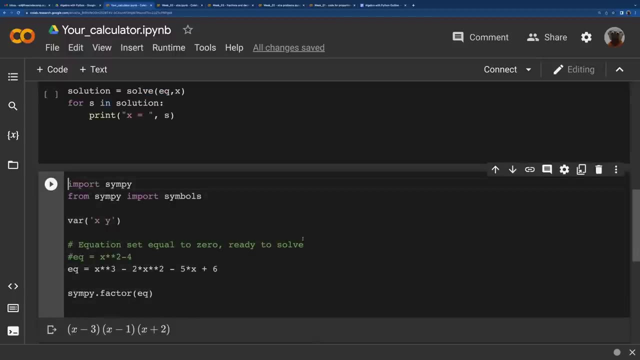 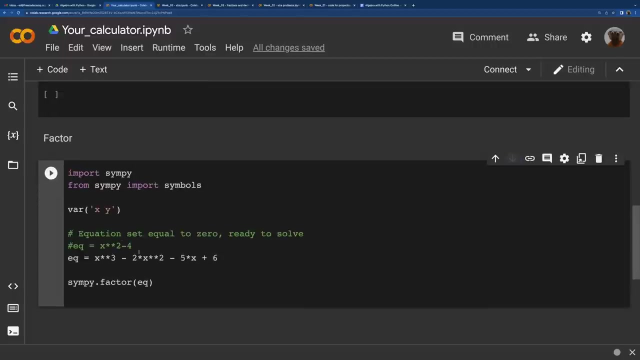 factor And down here then I will paste it. Oh, didn't show up where I wanted to. I can use the arrow move it down. So you know, there we go. We have set equation equal to zero. 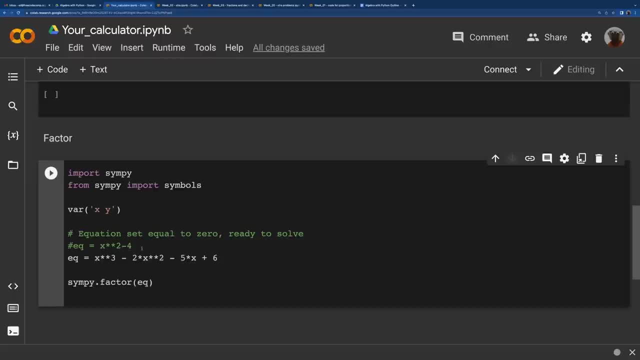 ready to solve. but we can even make this. you know equation to factor And see, you can put this however you want. There we go, And then you can factor things. So we have these, We can go into the next week. 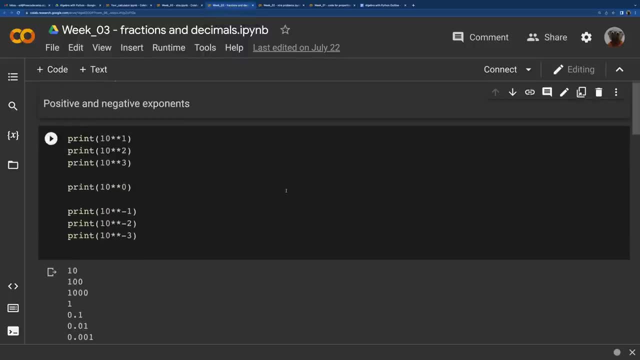 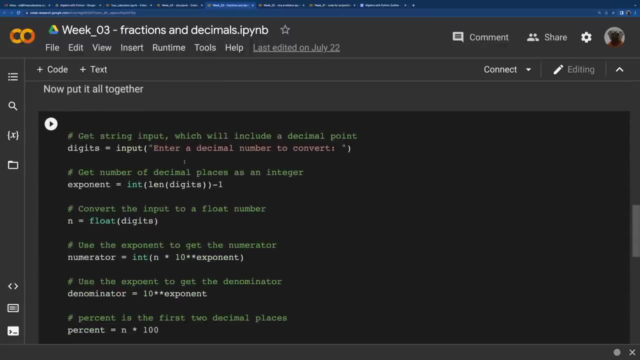 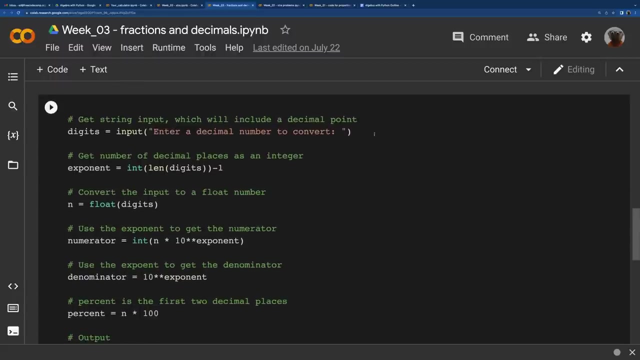 Now notice to put it all together, because when we went through and looked at some, some of these leading up to converting a decimal to a fraction, So this was putting it all together. You're prompting the person to enter in this. 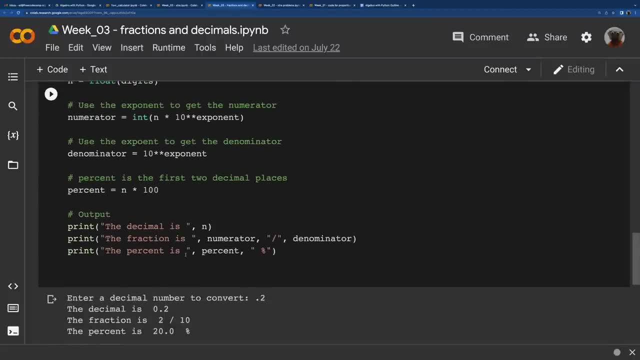 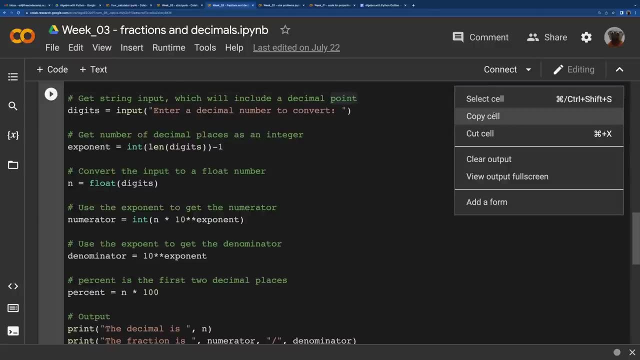 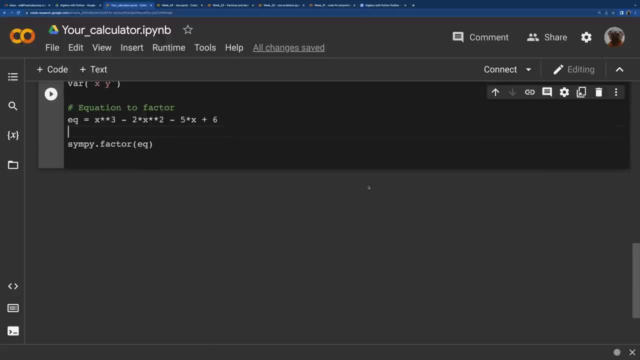 and then we're going to convert that output: the decimal, the fraction, the percent. So that's nice. Maybe we copy this And the factoring we'll get back to. So then we go down to here. Maybe I'll paste. 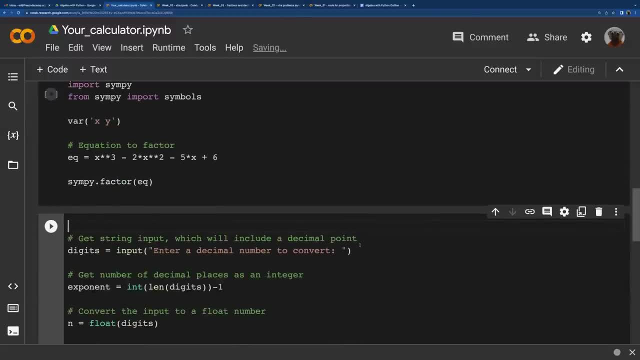 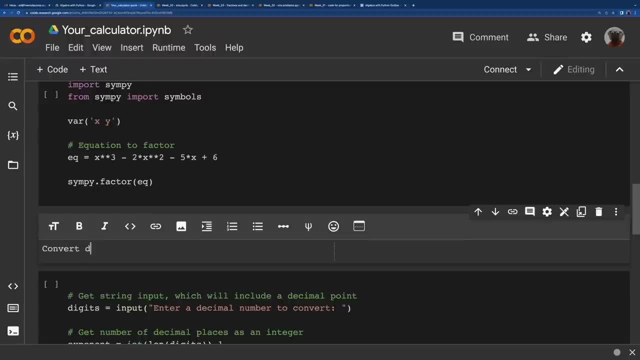 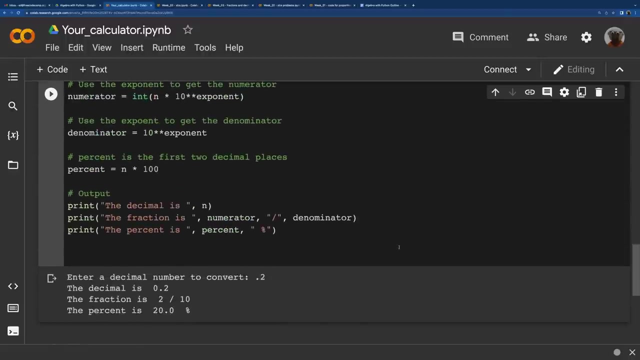 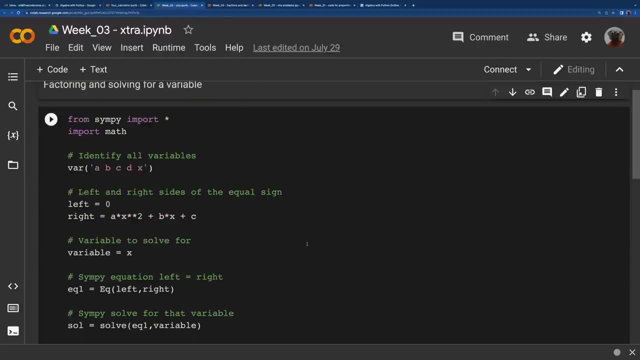 that here And that's good. So we just want some text ahead of it. Decimal to fraction. So you see, now you're putting together your resources here And we don't need that output right now. Now we have one more. 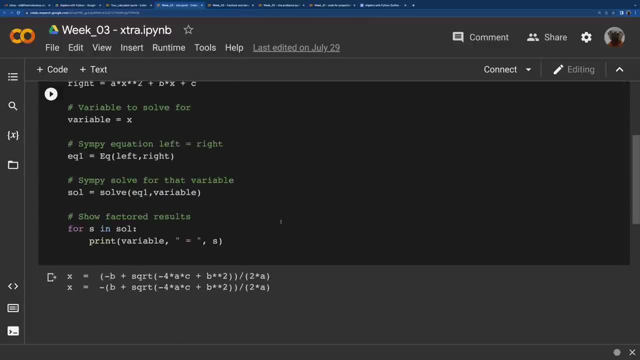 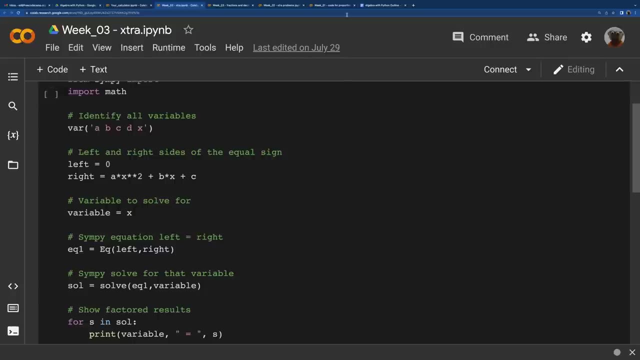 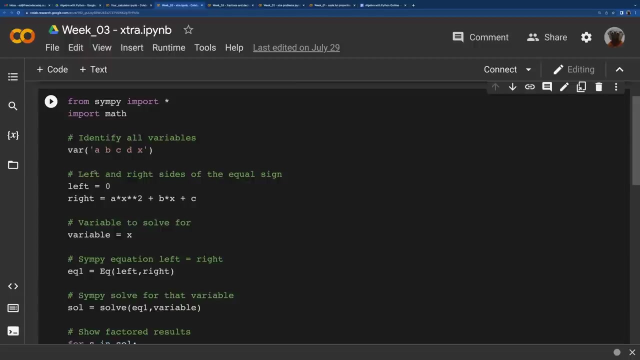 here Factoring and solving for a variable, And notice it's when I paste this. I might put it with the other one, But we see, remember we did this. Then you have the left side, which could be equal to zero. 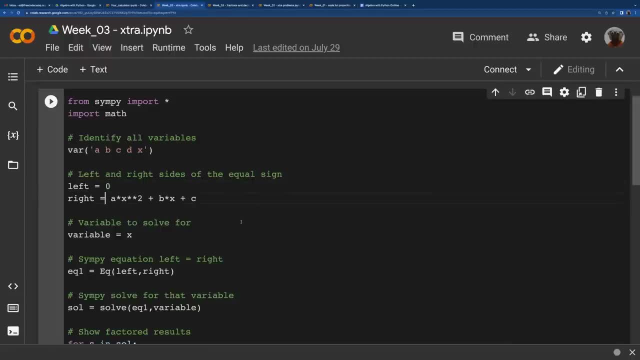 And the right side of the equation, which could be anything. You know, this would be about the only thing that you would need to change here: Change the variable you want to solve for, And I put all these as your basic common variables that you would 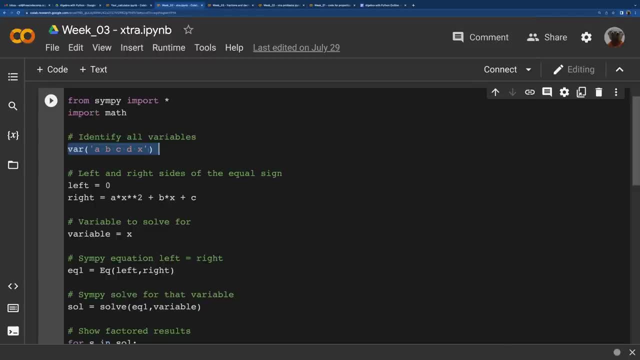 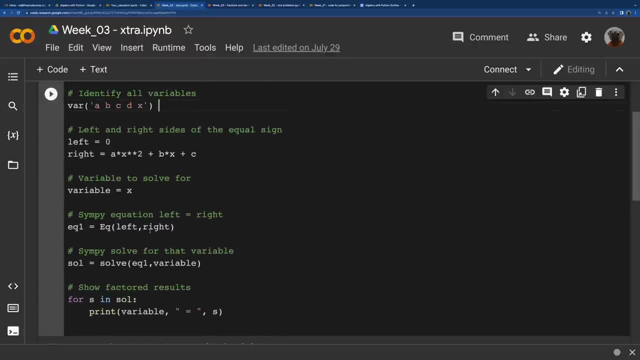 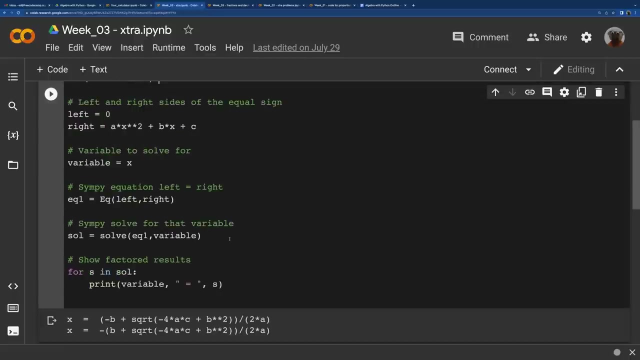 use. But you know, you could always change that too if you want. But you might not need to change that line. And then this one, we'll solve it, even if it is something that you can just solve for a variable, if it doesn't come down to an exact. 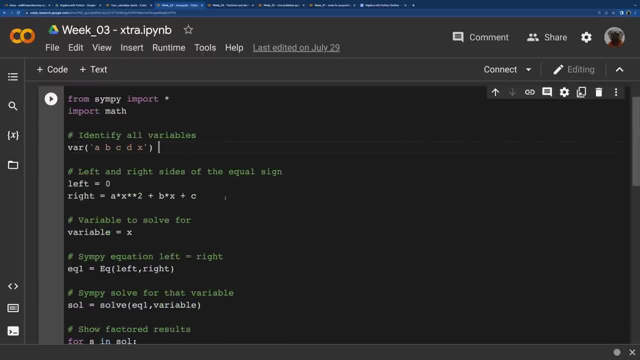 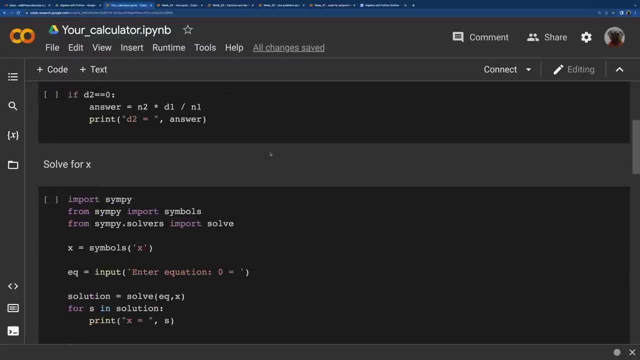 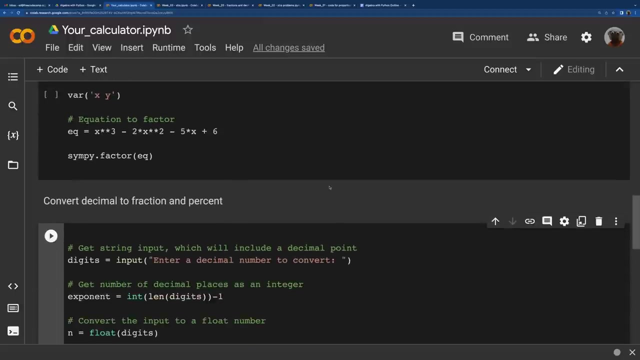 number here. So that might be a nice one. And then we keep this example in here. Copy this Now we might put this in here with: factor solve for x and factor solve for a variable. Maybe we put it in here somewhere. 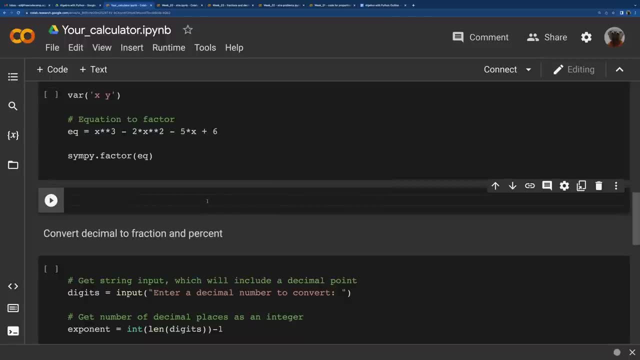 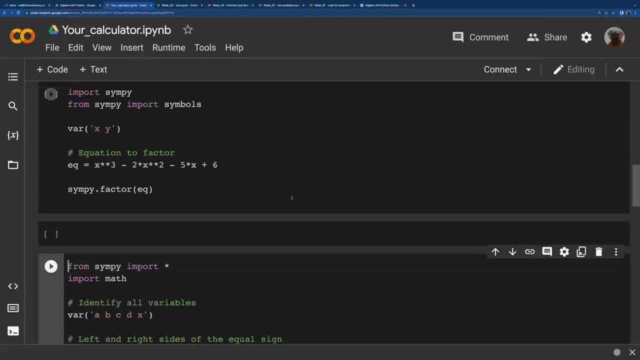 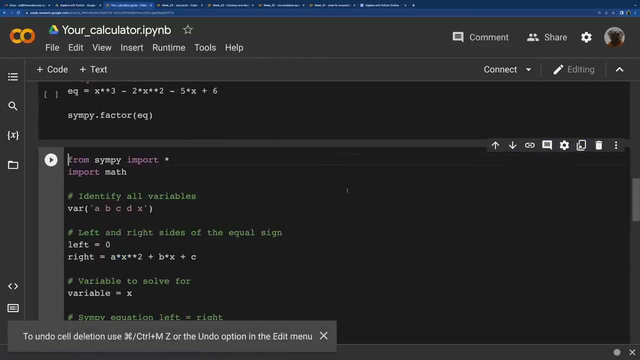 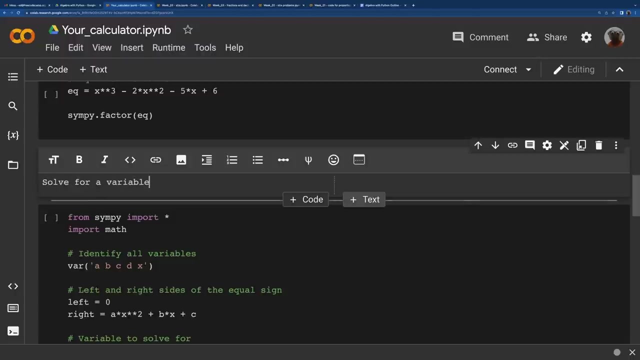 And notice you can just click and add code. I'll click right in here and paste it And this will be pretty much right where I want it to be. Then I might delete this. Add some text. Solve for a variable. Now, these are just. 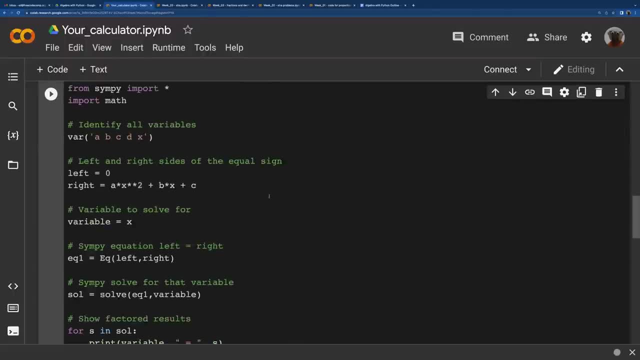 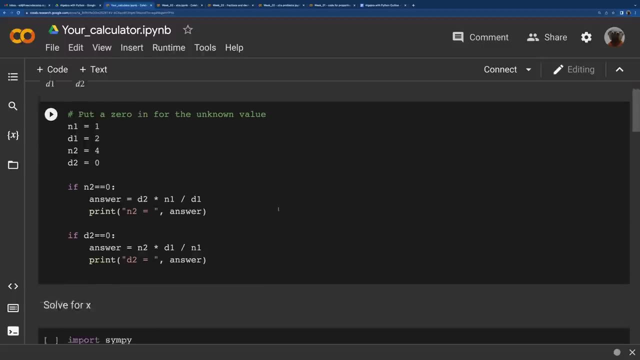 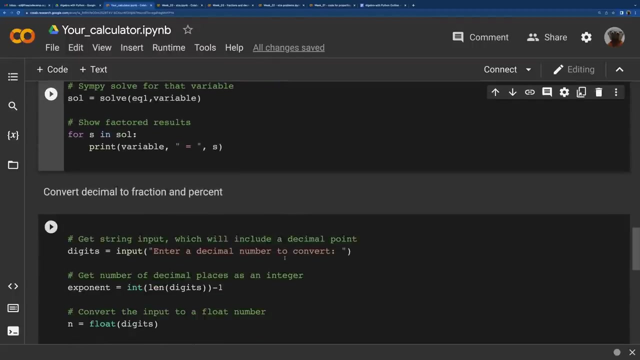 some examples here of how you could put this together. So then you have your resource here. Proportion: There we go: Solve for x Factor, Solve for a variable, Convert decimal to fraction, to percent, And then things that we do later. 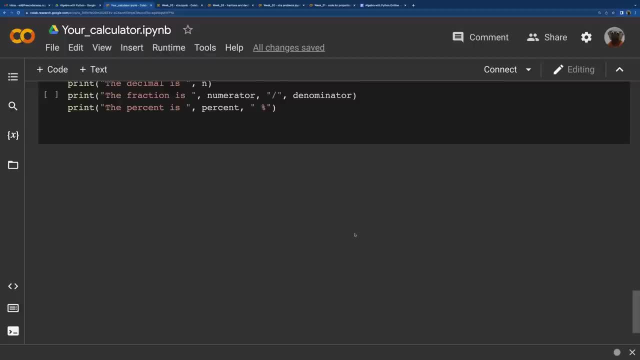 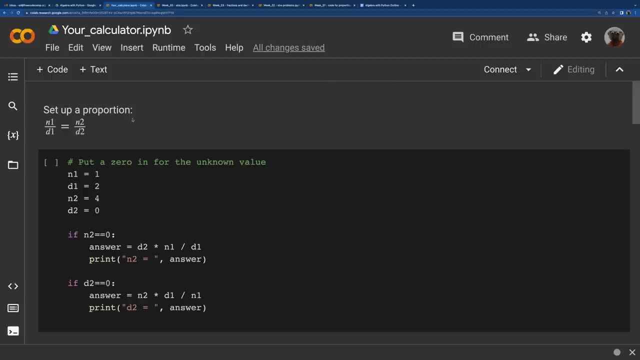 on. you could add more into this here Now, supposing you wanted to put a lot here and then you add all this. This is a lot of scrolling, So one of the things you can do is: now I'm going to start with. 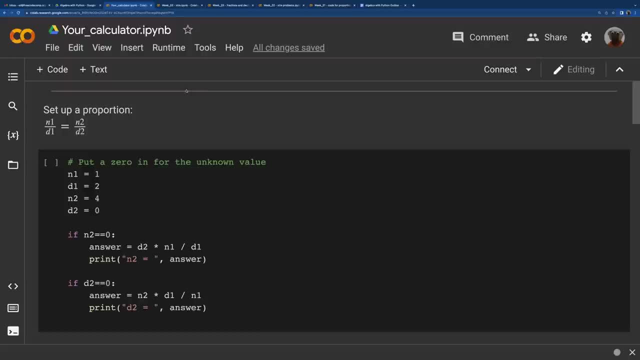 proportion I like. so right around here you could. there's multiple ways to do this. You could insert, You go up to the top, Insert, Insert Section header cell. So I'll do it one way. this way I'll do: insert section header. 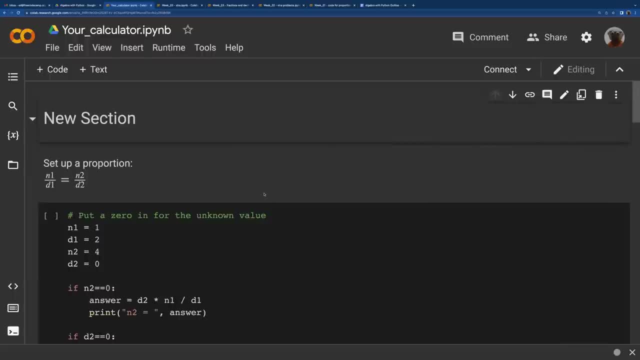 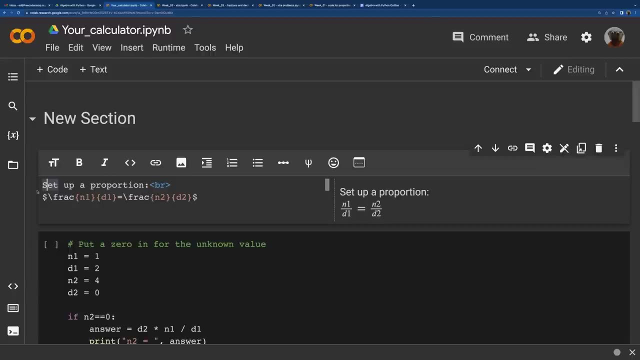 cell And actually I want that above. So, and notice this, when you double click on this, you see some of this, These text boxes, except HTML. Look at that. The BR to split the line And they accept latex, which is how to format. 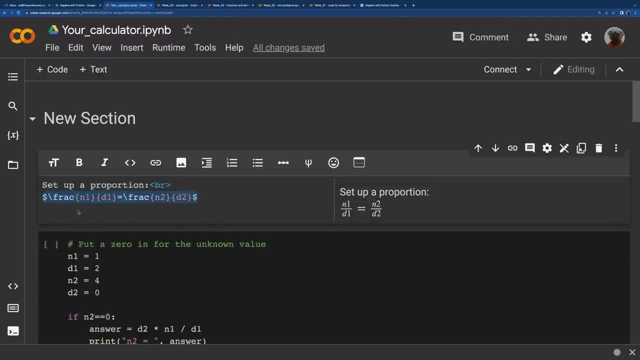 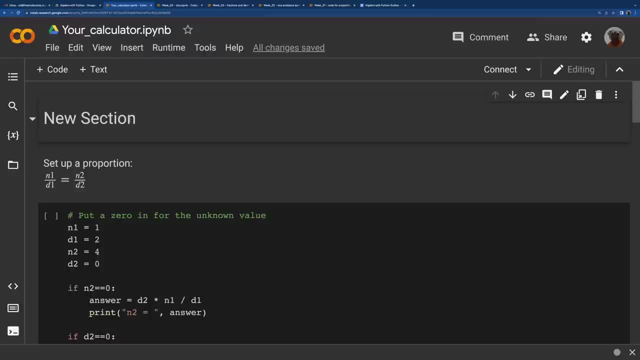 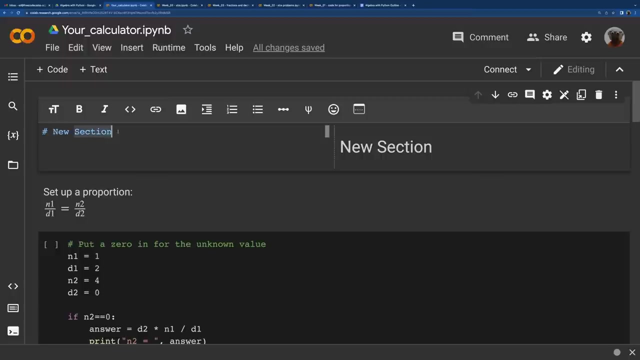 various things: Fractions, formulas, all kinds of things. So in this new section- and you see, because it's in this text part, that's not a comment in Python, It's the new section And I might just make this proportions: 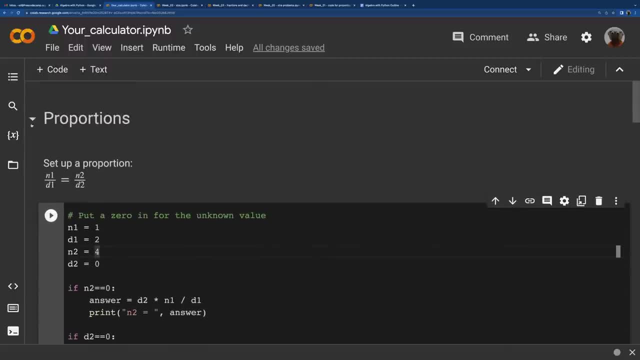 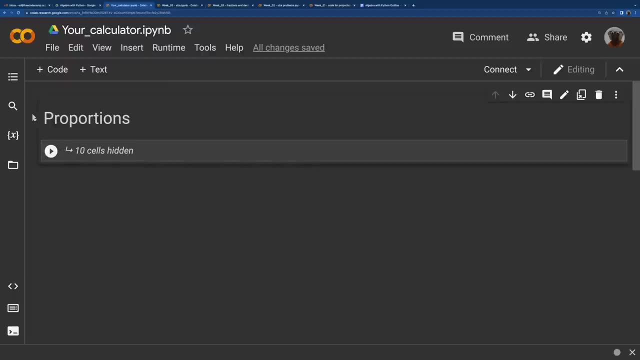 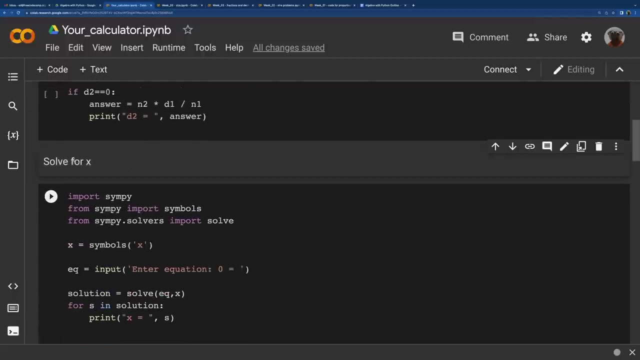 Okay, So now you see, it takes that and all these cells become a part of that section. I don't want that, But what I want to do is if this next one, I want to make this the section and I don't need another one. 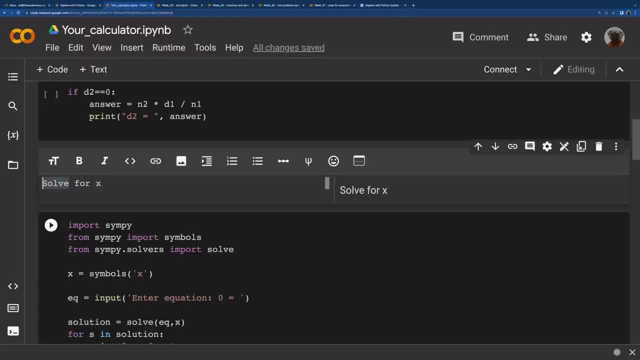 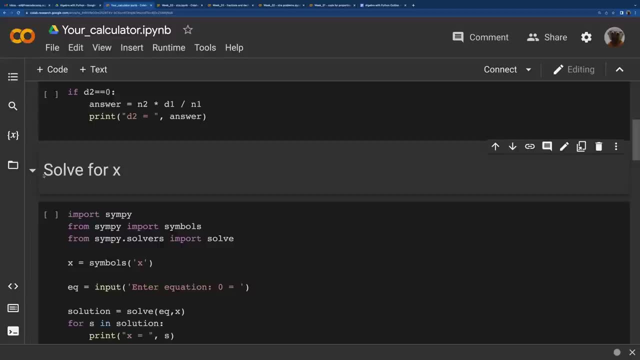 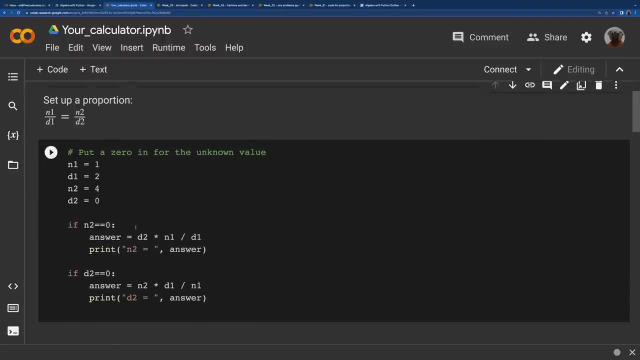 I think that'll be the section header. There we go, So I'm just going to put this here. Now that's a new section, So we see proportions now just has the two cells, The text about setting it up and then the code. 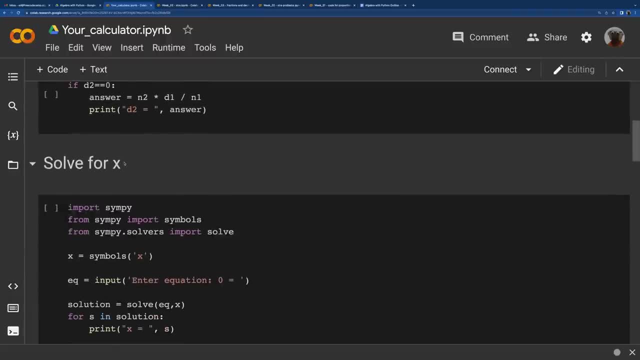 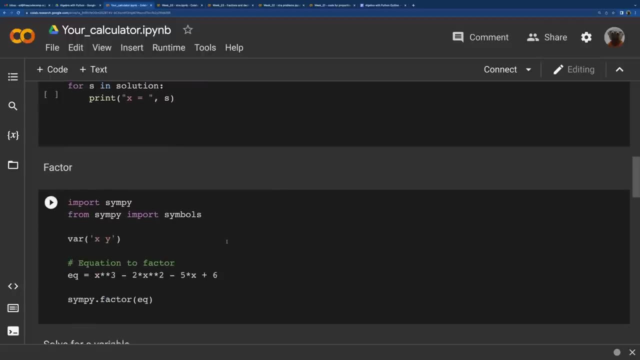 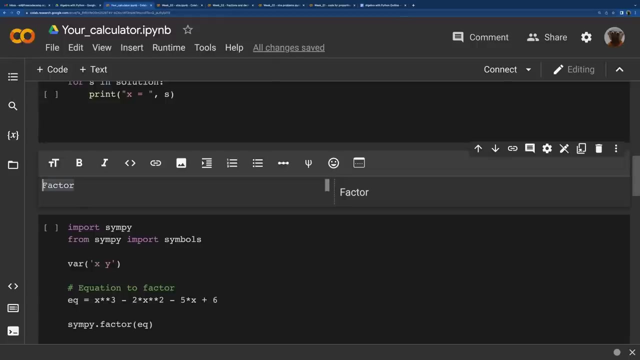 And solve for x has just one cell, because that section said it all, and then we have the code. There we go, Factor, And maybe you want to say something more than just factor, but you can make this a section heading Solve for a variable. 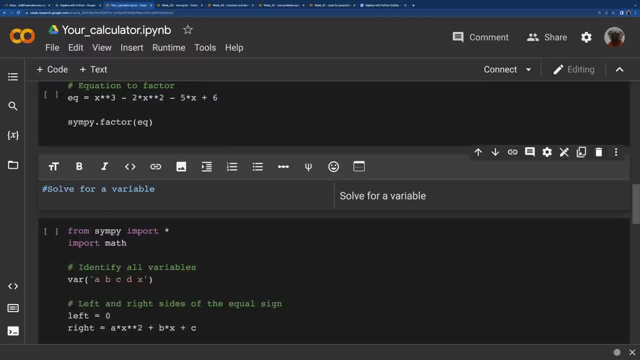 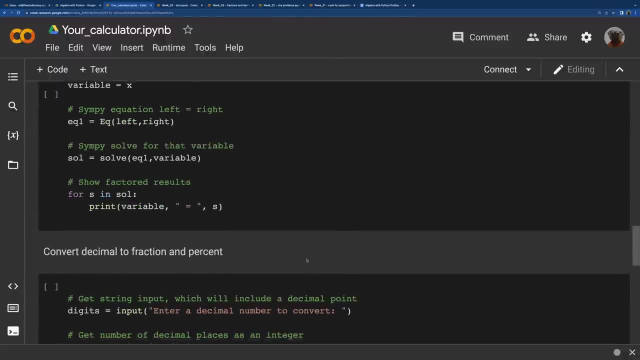 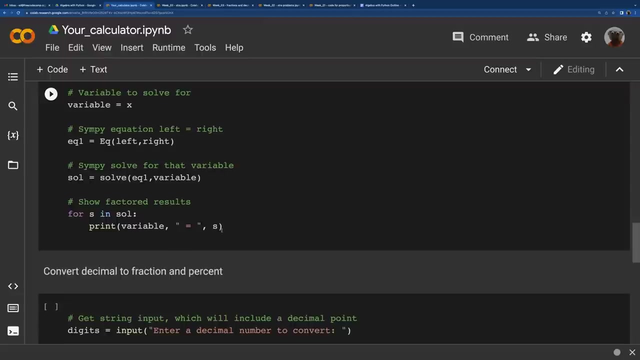 There we go And in seeing all this together. So you see, solve for a variable. Convert decimal to fraction. You know that probably I didn't need anything else here. Solve for a variable. All the rest was explained in the comments. 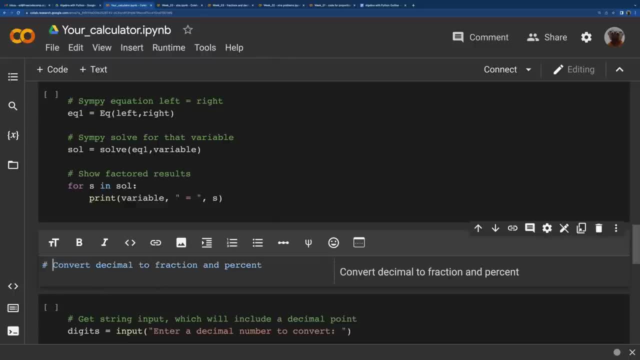 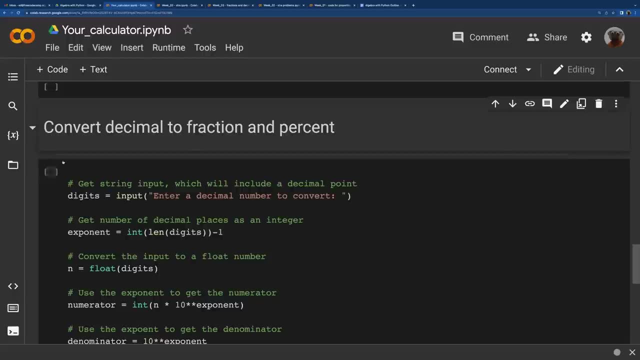 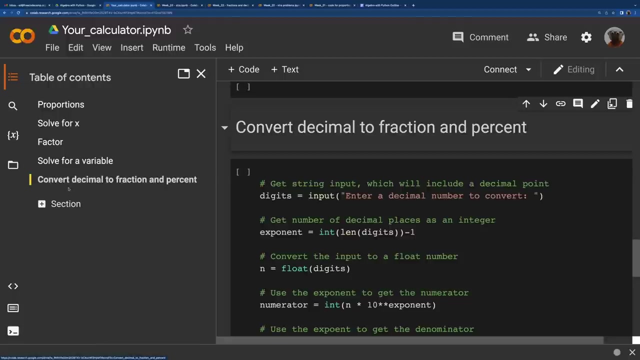 And convert decimal to fraction. So now this just has the one cell, And the advantage of doing this is over here. you see these lines, Now we have the table of contents here. There we go, And I could change. you know, that's long enough. 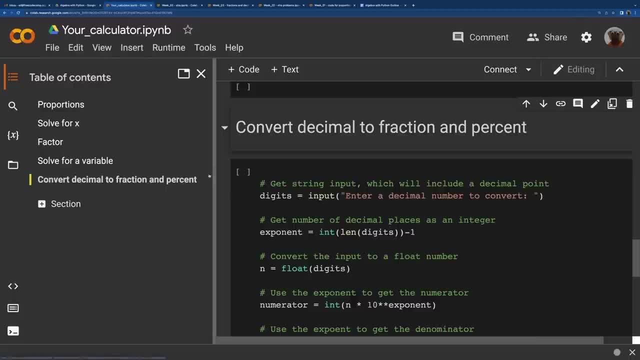 I don't like it when it goes on to two lines, But that fits, so that it's a longer title, but that's okay And you can have your table of contents that you can actually go through and you see, jump to proportions. 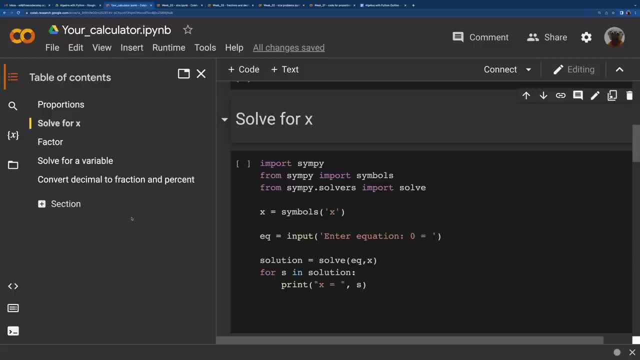 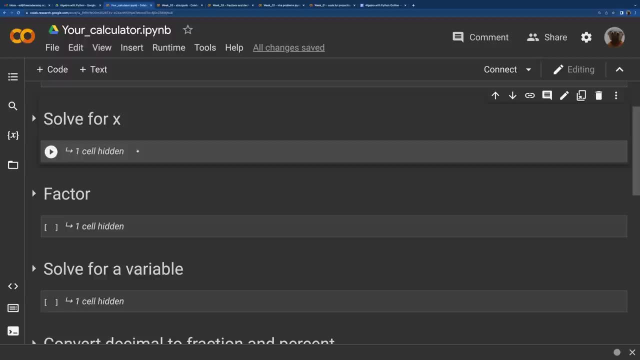 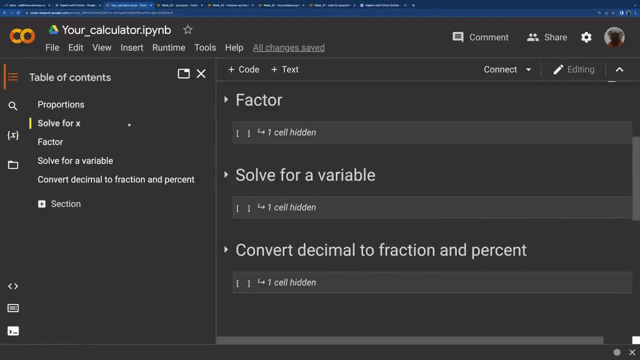 Jump to solve for x. You know different things And in the view you could change the view to collapse sections. You don't have to, but you could. And then you see you have all these. So these are some things you can do in putting 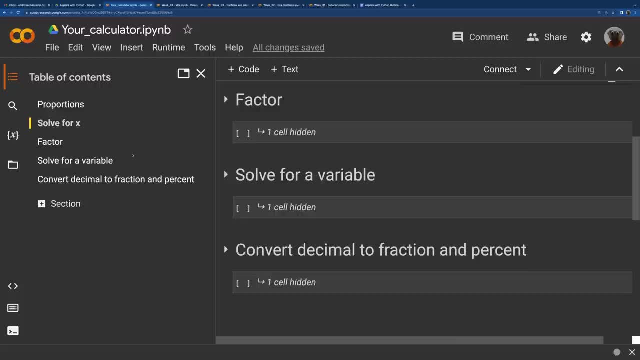 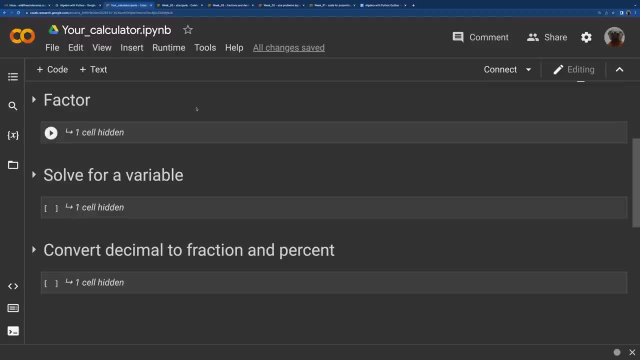 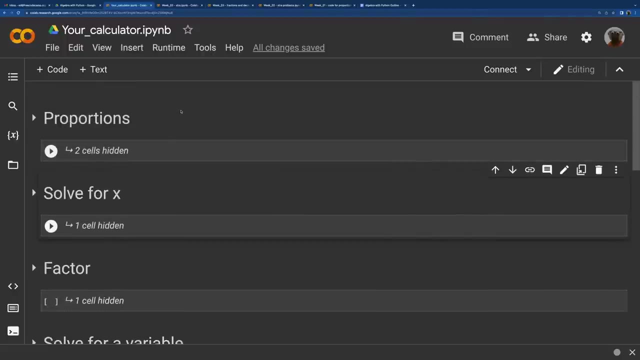 together your Google Colab notebook. You know I want this to be your calculator that you're building, So then you're learning how to do all this, but then you also are building your resources here that you can then refer to. Oh, what do I? 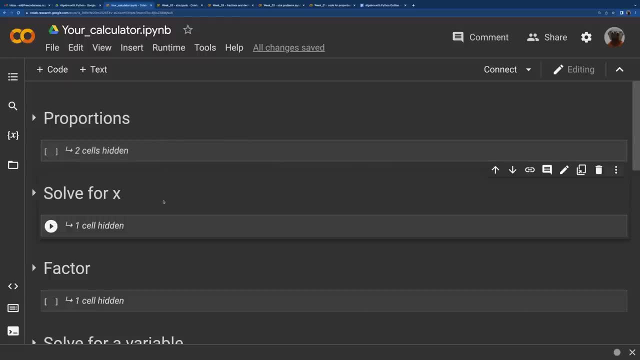 need to do, Click on it, Enter what I need to enter and solve it. You know you're essentially making your menu here, So that's what I want you to do for this unit is take a look at what we've been doing so far. 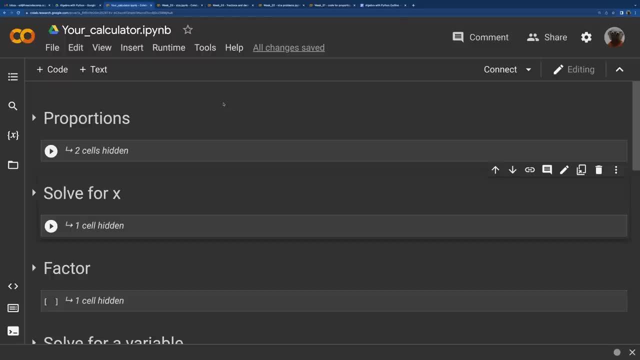 and put it together in your own notebook. Some of the things we'll do later will even get fancier and we'll make some of these into functions that you can use in different places, But this would be a good place to put together your notebook of resources. 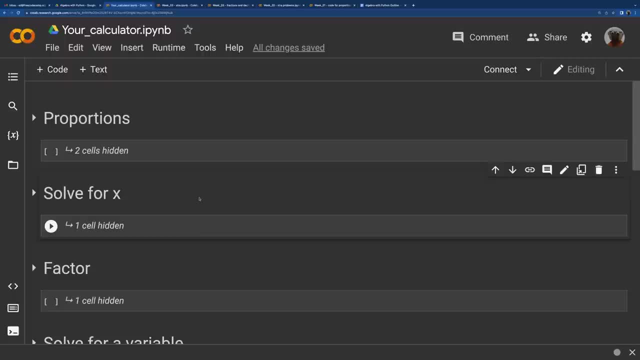 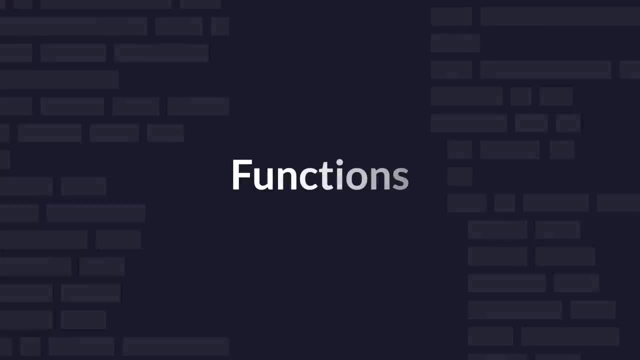 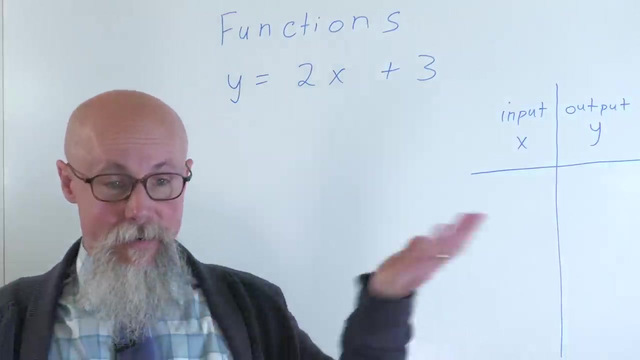 Here's one way to do it, but you can tweak it to the way you like it. Alright, And now we're ready to learn the next thing. So what does it mean to be a function? A function means it means, in math and in code, that you're. 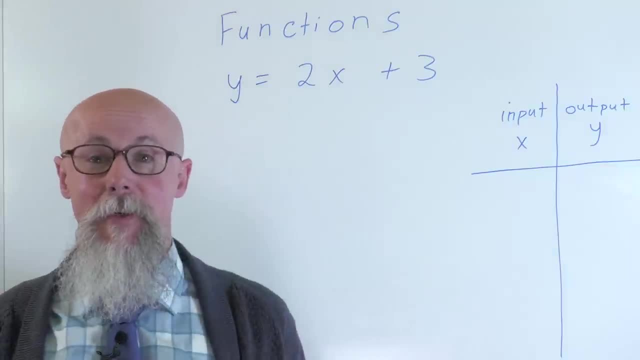 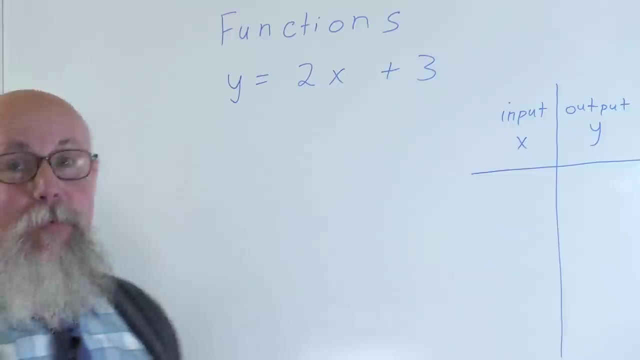 taking some input and then doing something to it. And actually there are some functions in code you don't have to take input, but in math we will. So, like we were talking about our unknown number being x, the output will be y, So each function. 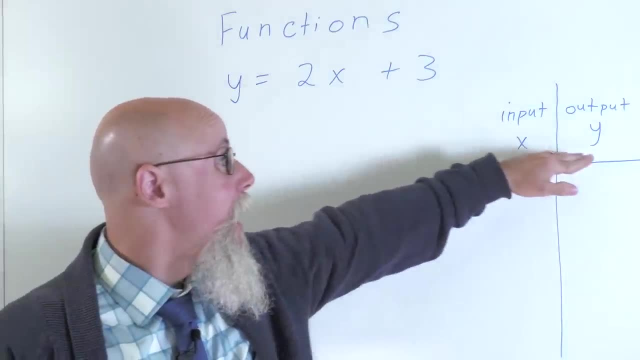 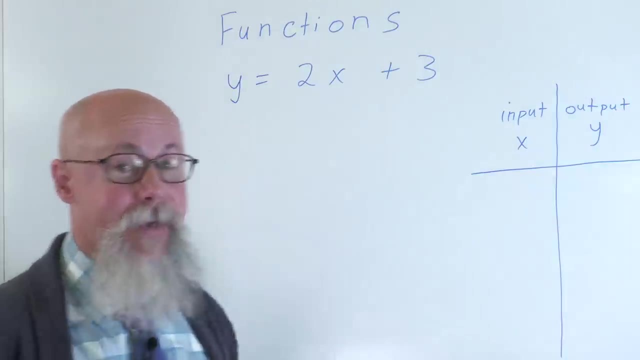 we want to take x as the input and then we're going to say that the output is y, And here we're dealing with all numbers. What am I doing to x And then outputting y? So you see, we have like solving for x we were doing. 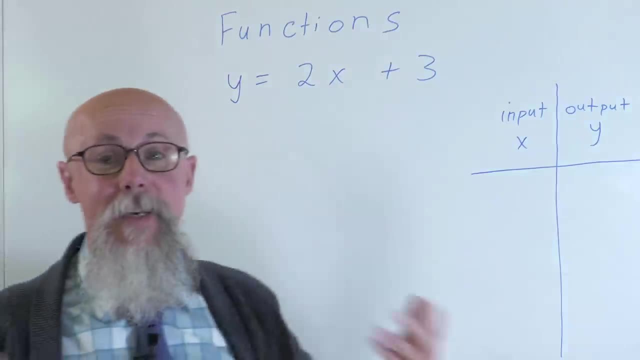 before. but now we have a second variable And we still want the idea that, just like in the alphabet, x comes before y in science and in research. we can call x the independent variable, because that's what changes first And then y is the dependent. 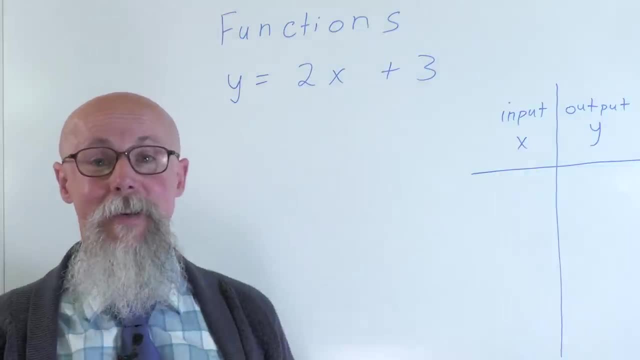 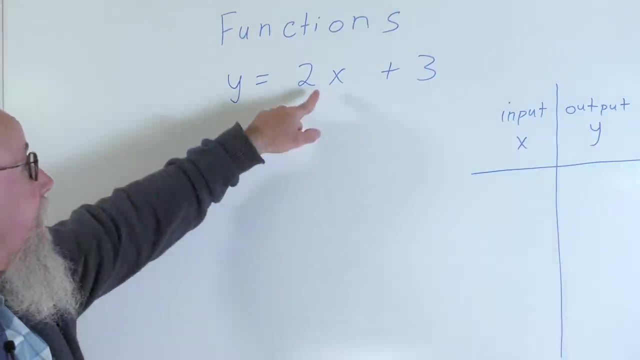 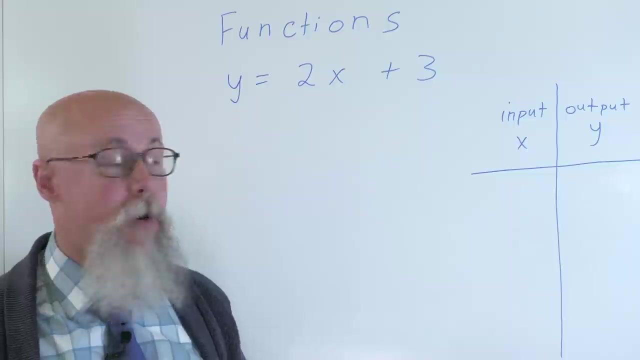 variable because it depends on what x does. So if I want to solve this or do anything to it, then I'm going to plug in a value for x And I can pick any value. I might start with zero, So I'm going to define it over here. 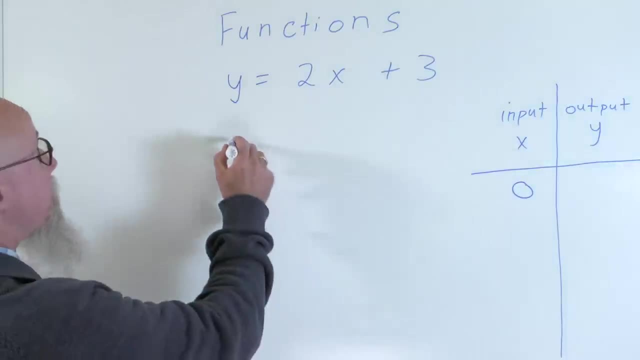 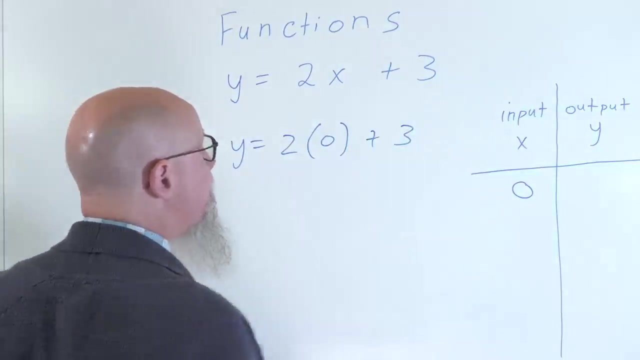 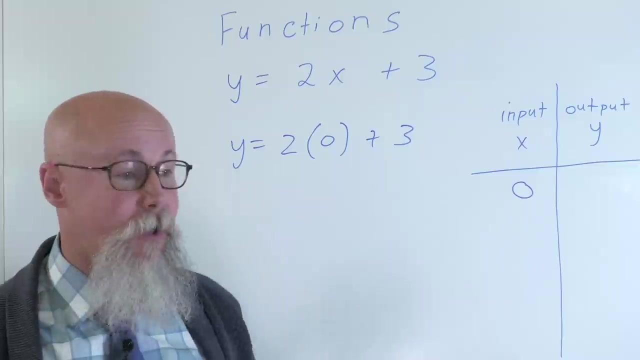 My input x is zero. And then what happens when I plug that in? So that would be: y equals two times zero plus three. And you see, I'll just put in zero in parentheses where I plug in this number, because it highlights that that's what I. 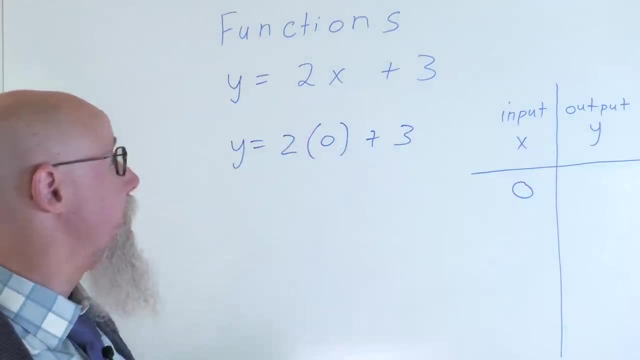 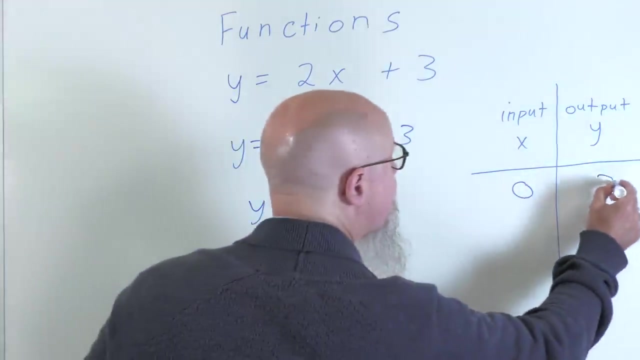 just plugged in, and also the fact that they're next to each other. I'm still multiplying. So when we do this, two times zero is zero plus three, then that would be y equals three And my output is y, And if you remember, then that's. 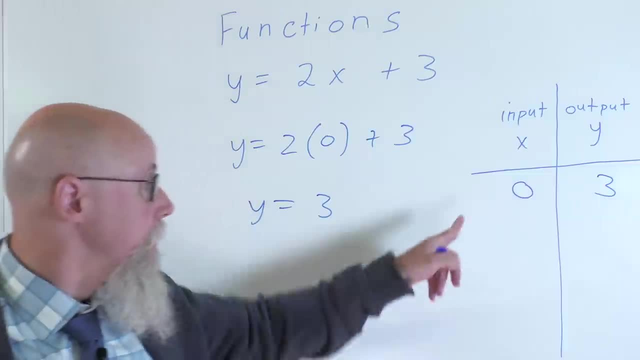 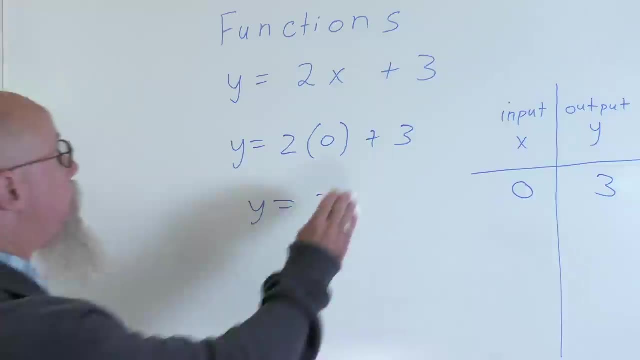 an xy coordinate on the graph. x is zero, y is three, and I'd be able to plot that point. And I can keep going. What other points can I? what other numbers can I plug in? I'm even just going to keep this. 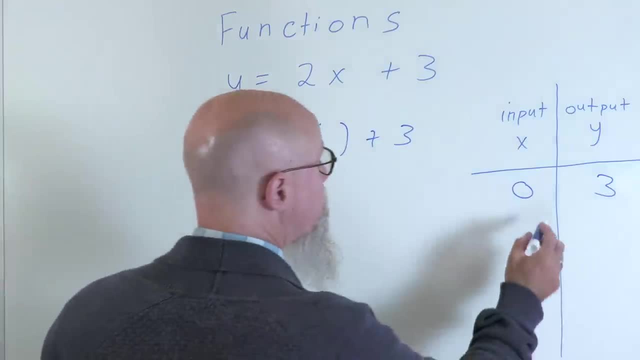 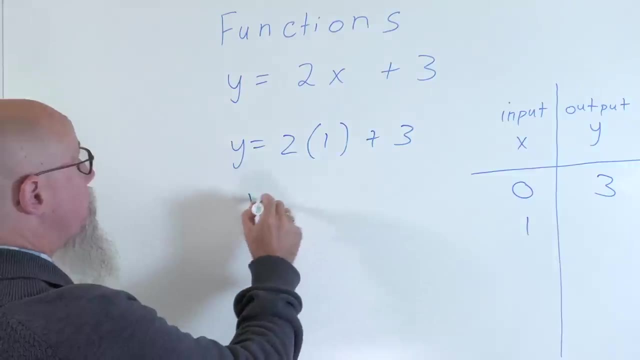 So, supposing I have x equals x equals one, Plug in one. Two times one is two plus three is five, y equals five, And then we'll plug that in, And I can plug in as many or as few, I don't have to have integers. 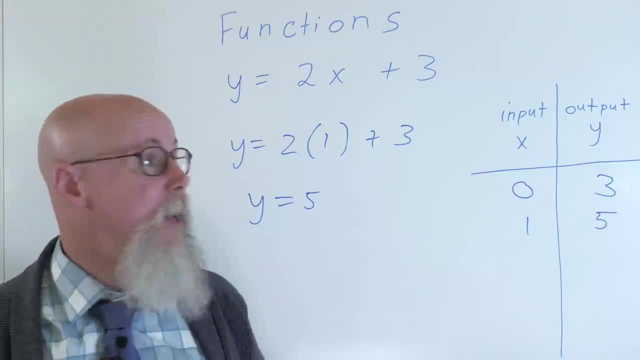 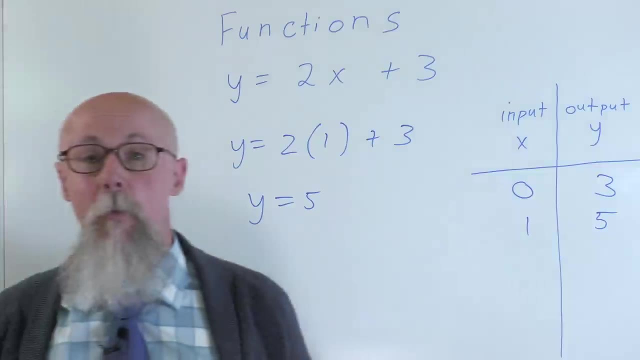 I tend to do that so you can see the numbers a little bit clearer. But you know you don't have to worry about doing any other calculations in your head. But if I have this, I can put in whatever numbers I want, As many or as few. I can put decimal numbers. 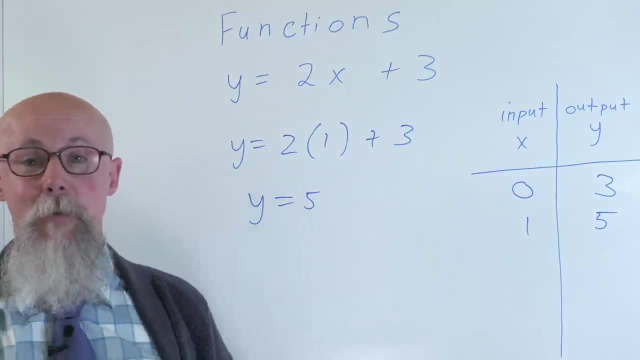 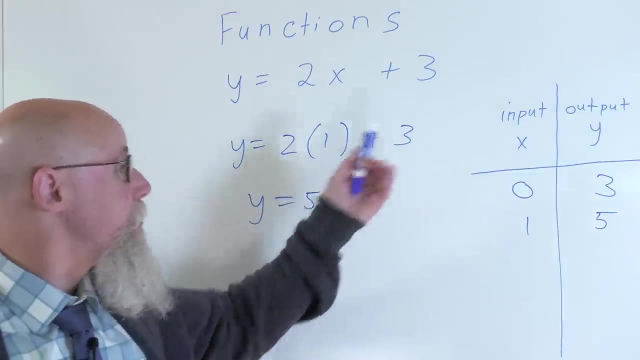 in there And we can plot these on the graph, which we'll talk about a little bit later. But this is the essence of a function: That x comes before y. I plug in an x value and then output the y value. So 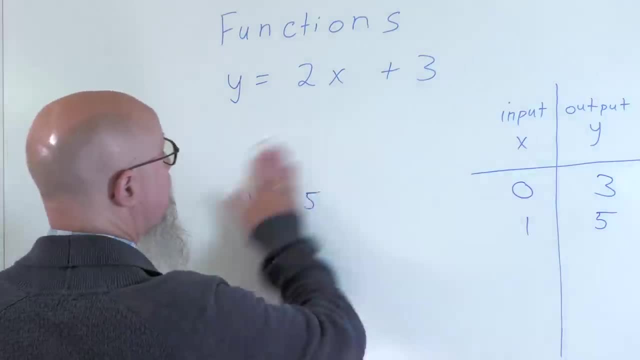 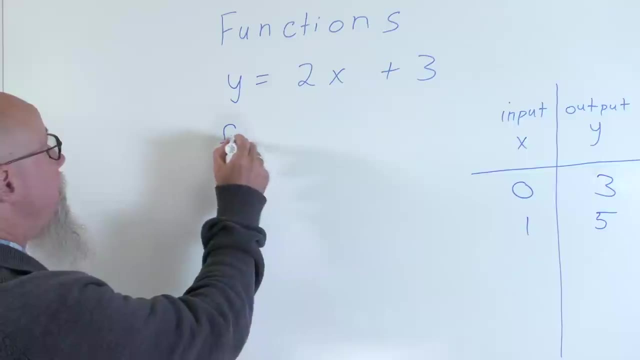 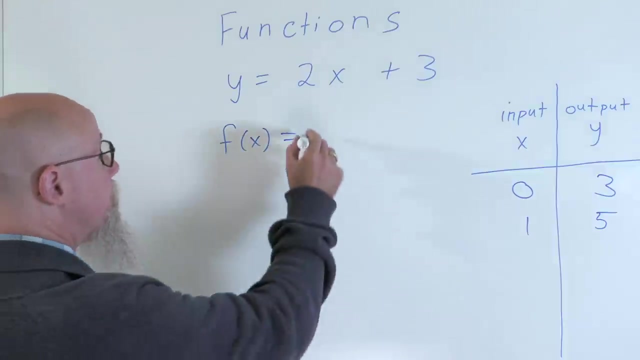 another function notation that a lot of people like is, instead of using another variable, y- and this connects a lot with the way the code's going to look- We call it f of x and f for function, So 2x plus 3.. 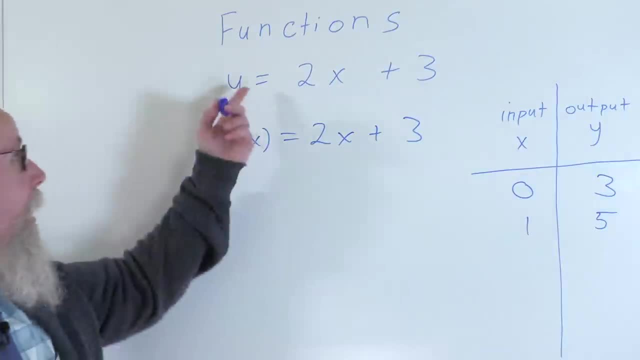 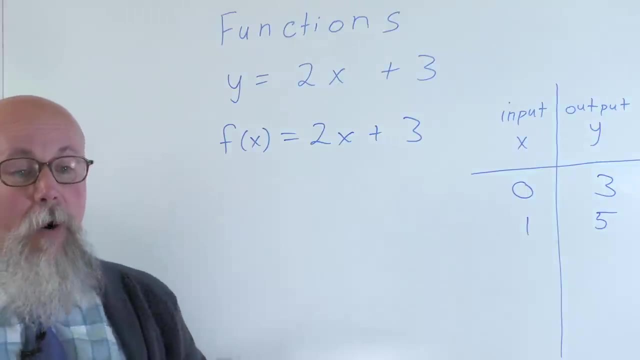 So, if you see these, these are the same thing: y equals 2x plus 3, or f of x equals 2x plus 3.. This notation f of x, and that's where we read f of x, f for. 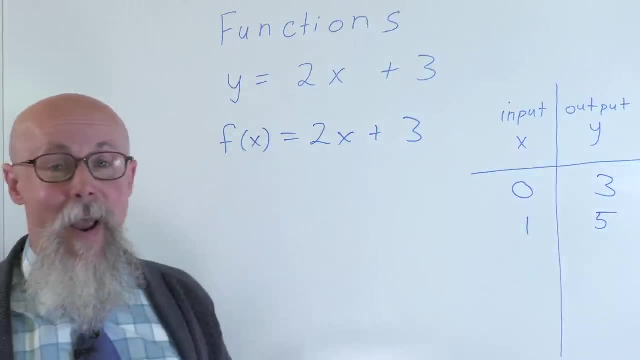 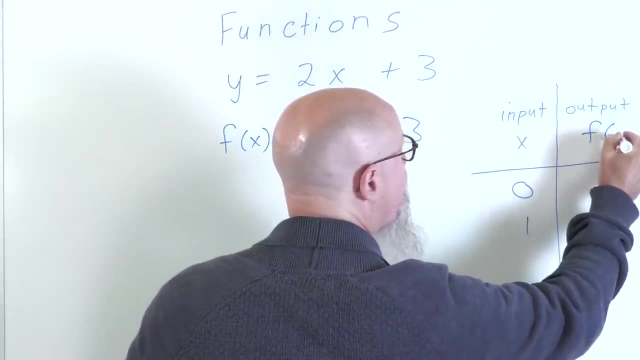 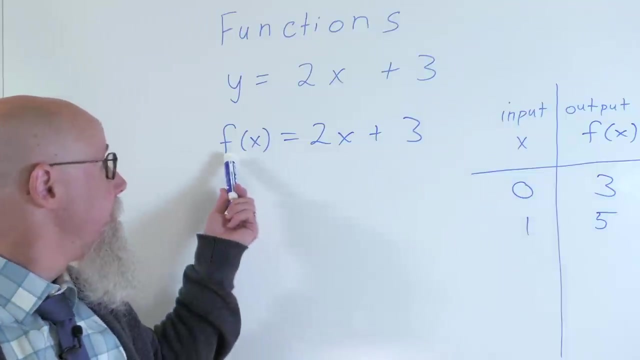 function. We solve it the same and this connects a lot more with your computer science. So if I have the output called f of x, one of the advantages when we get into writing the code is that in algebra we tend to just say f for function. 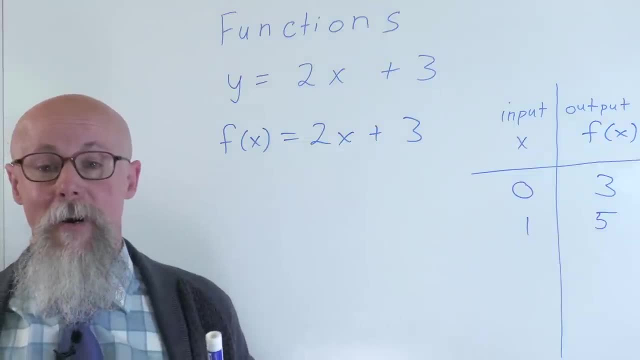 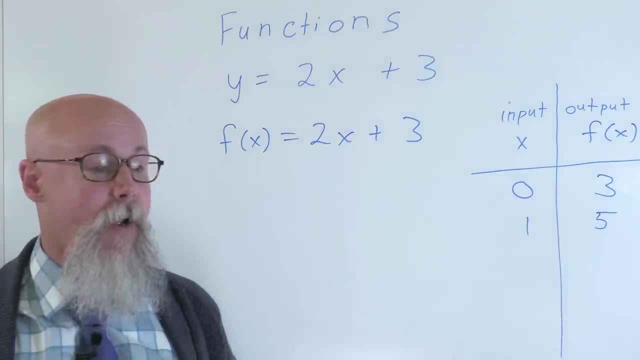 But in writing Python or other code you can actually give your function a name, and it doesn't have to just be f for function. It can be add, divide, calculate the area, something really even a long phrase like that, as long as 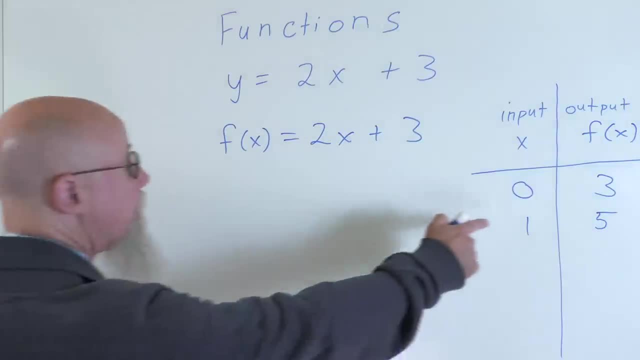 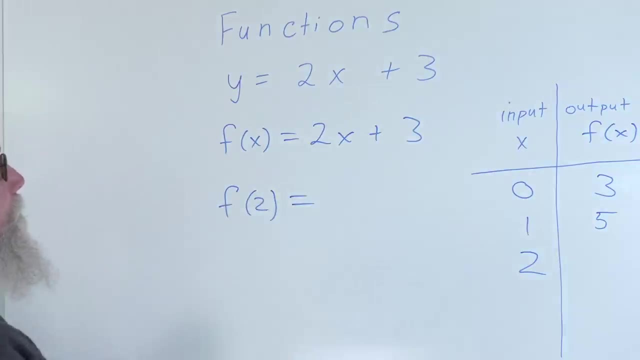 there's no spaces. So if we have this and then sometimes then let's say, if I wanted to plug into 2, I could write in f of 2.. And so again, the usefulness of this notation is because I see what am I already? 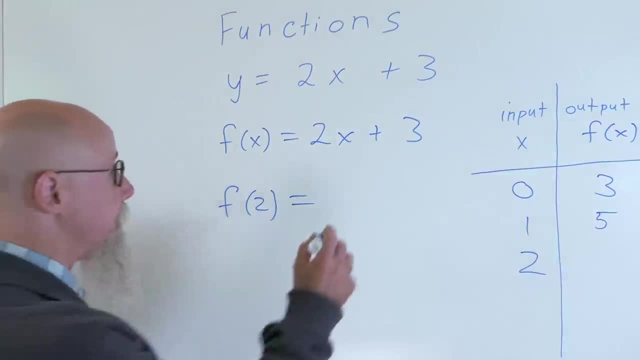 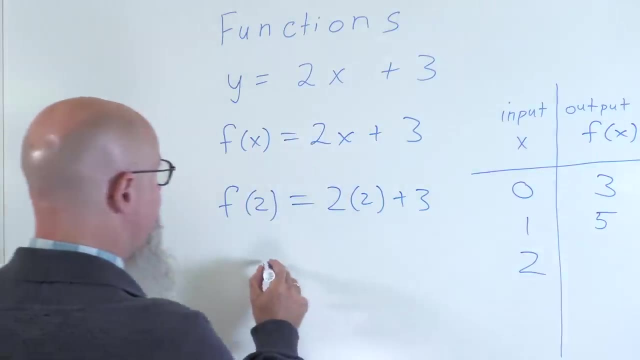 defining as my input. And then I know what am I doing next. I'm going to do 2 times 2 plus 3.. 2 times 2 is 4, plus 3 is 7.. So f of 2. 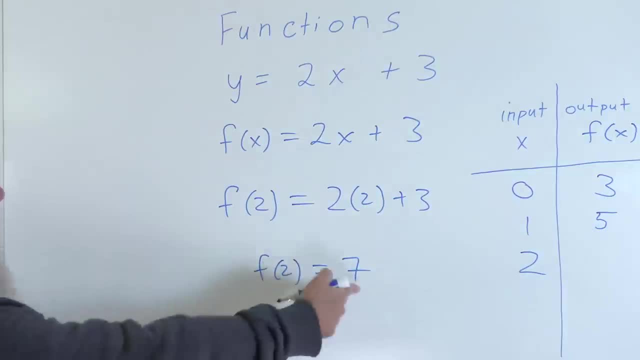 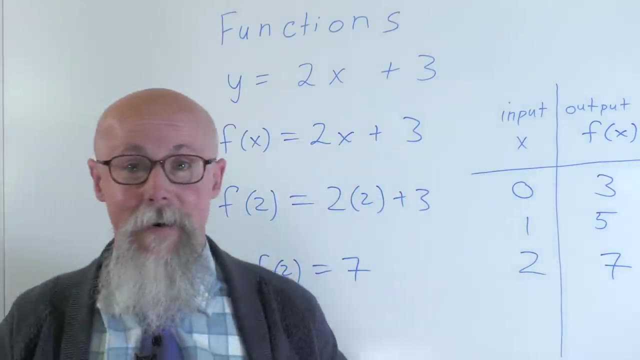 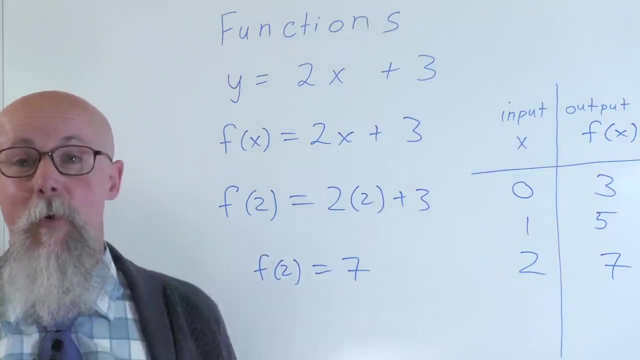 is 7.. So now I know that answer and when I see that x is 2, y is 7. And we'll see how this really relates to the code and how we can write even a little bit more elaborate functions with code and how we can. 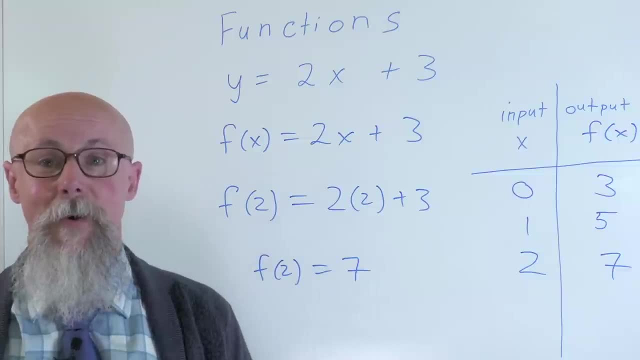 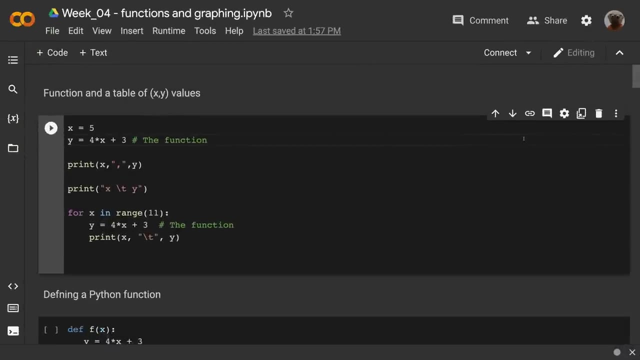 define the input there, Then we'll look at graphing it. Alright, so let's take a look at the code. So with the code and functions we can do very similar to what we would be doing by hand writing out the math. 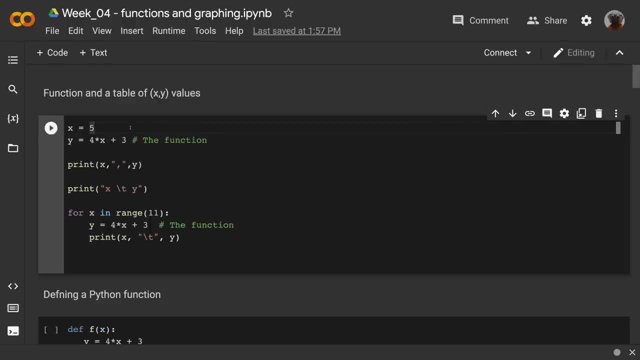 Here I'm just going to define one x value as an example, and here is the function that y value y equals 4 times x plus 3.. And you see Python syntax. I have to make sure we put the times So. 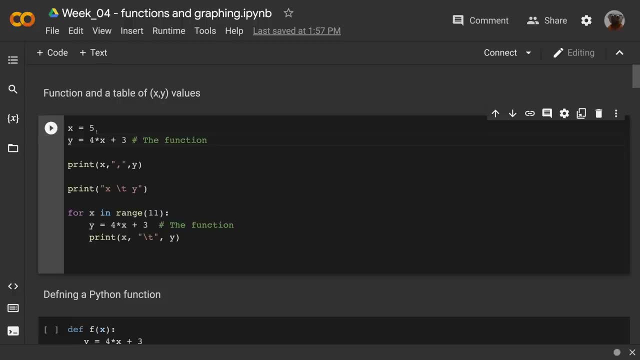 I'm just going to plug in that y, x value become, you know, substitutes in for this x value. so it's 4 times 5 plus 3, and then I'm just going to print out my solution: x comma y. So we see that. 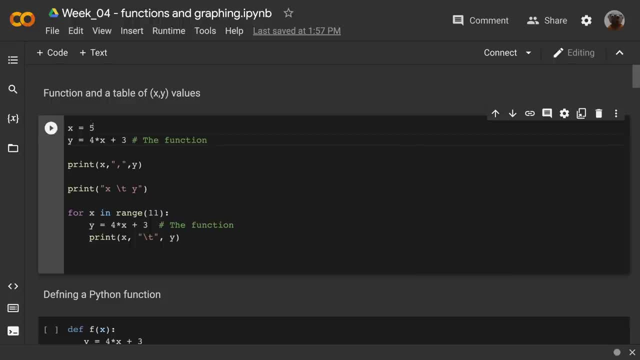 And before I print that out. so that's one thing, one x value, but I can loop this. So I'm going to print out this line here, which is x, and then I'm going to put a tab y. so 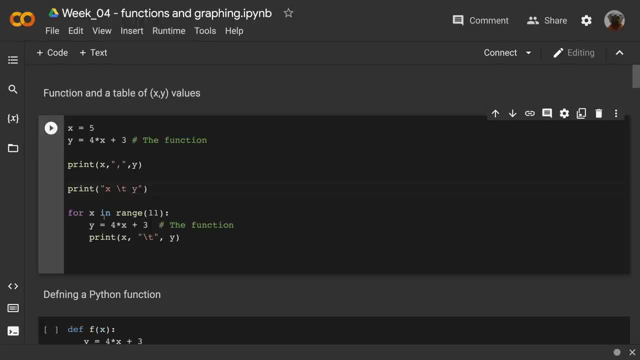 that's defining my columns here- x and y- and then what I'm going to do is loop through all those values. So for x in range 11, so x is going to go 0 through 10, and then I'm going to take that same function. 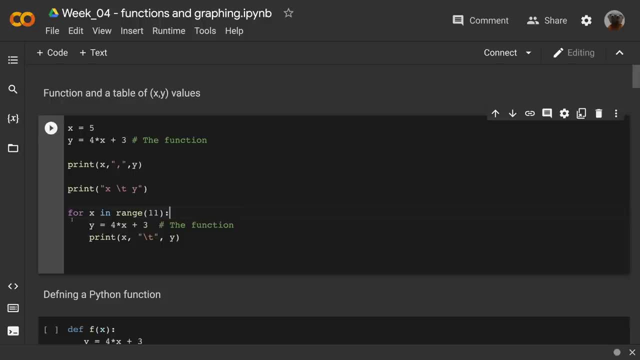 and each time then I'm going to plug in that x value, solve for y, and I'm going to print out the x, y values And in this case again, I'm going to put the tab in between. So this is the essence. 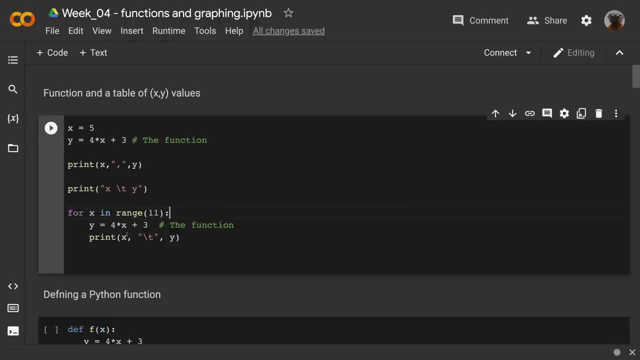 of what we're doing with a function. Each time I get an x value, plug it in, solve for y and then I have an x- y value and this is going to print this out as a table. So when I run this, 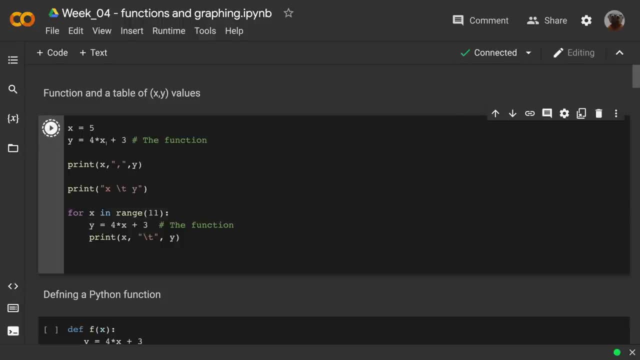 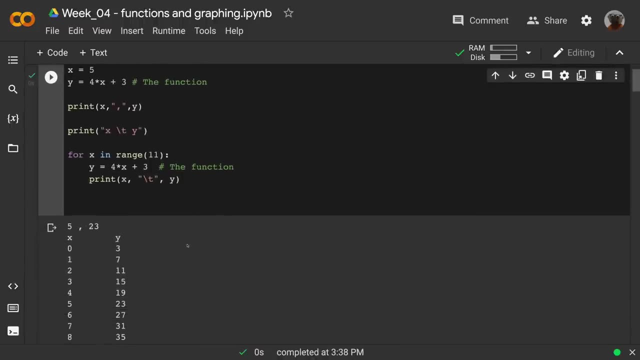 we'll see it'll come out. first of all we'll have that one solution, you see 523, comma 23,. that first solution, and then we have our table x- y and all of our x- y values. 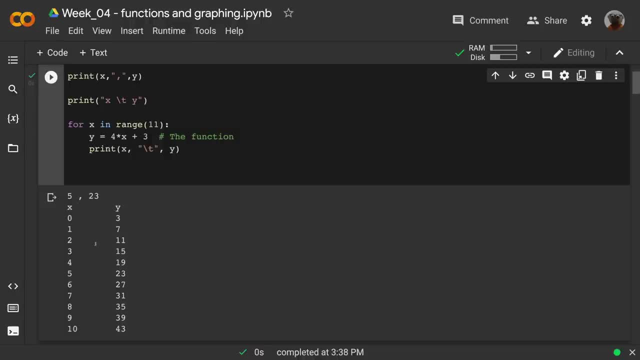 If x is 0, y is 3.. If x is 1, y is 7, etc. And we also have 523. that shows up on the list too. So that's defining a function. Now, Python has a lot of other functions beyond math. 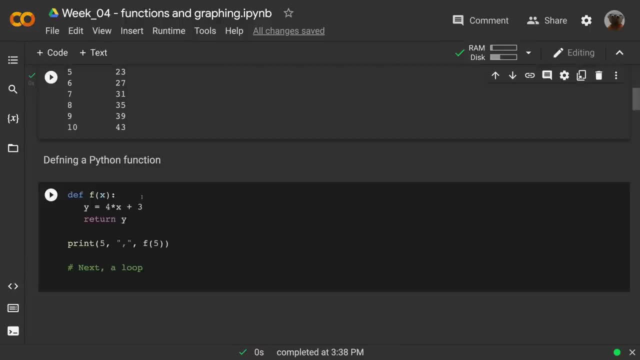 you can do things with, and we can still use that same type of Python function definition for our math. Here we can, on this line, define the function. so def space and Python. I can name my function anything, but I'm going to use the classic math. 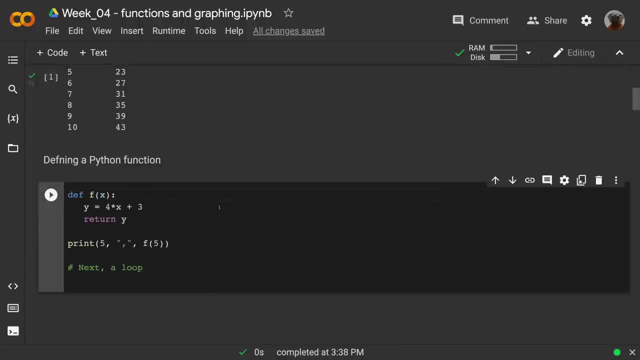 notation f of x. And then here I have the colon. so this is going to define the function. Everything underneath is indented 4 spaces and I have y equals my 4 times x plus 3, that's the function. And 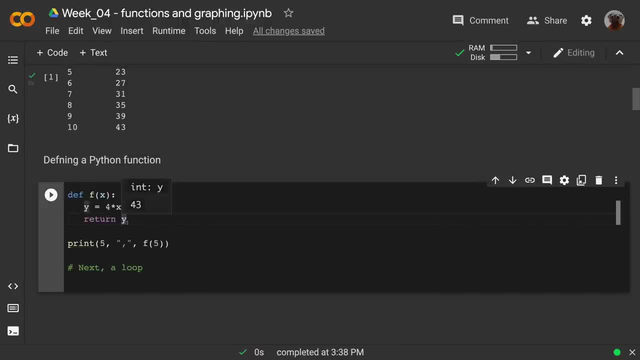 what am I going to do? Then? I'll return the y value. So whenever I run this, that'll return the y value. So you see this in use If I print here, if I print 5, so I already know I want that to be my x value. 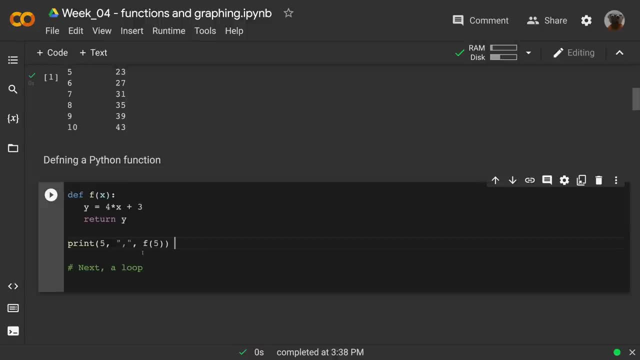 comma, and then I'm going to call this function right here f of 5, and it's going to take that and run it through. there we go: same type of thing, um, same type of thing. then we'll um. 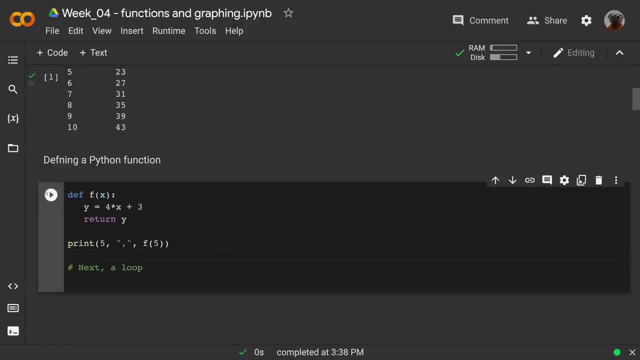 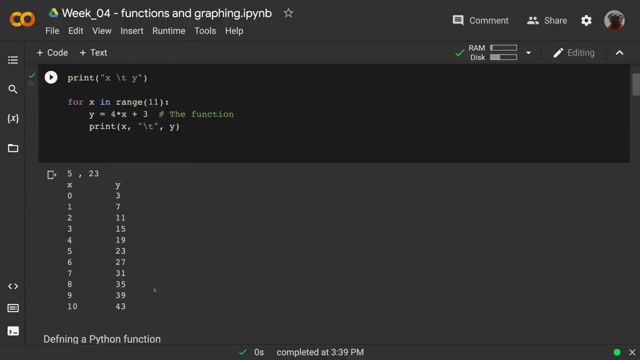 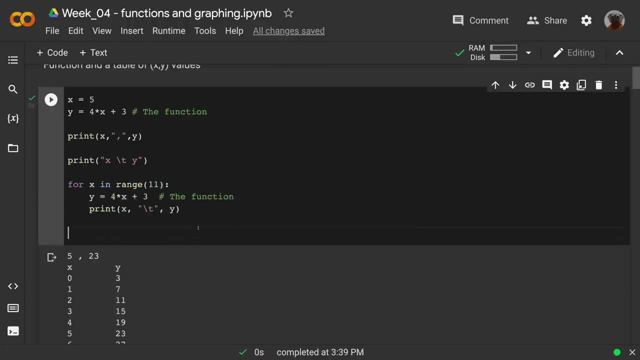 define this, and when we run this, it's just going to print that 5, 23.. And next we could put this in a loop. I could just take this same loop here and I'm going to copy this, and I can just take that same loop if I wanted. 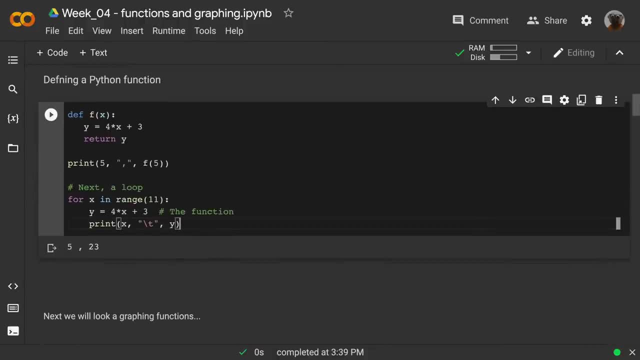 to, and in this case I'm going to print, because I already have that function defined. I don't need this, and I could really just put that here. f of x, You see, so I could just have right here um. 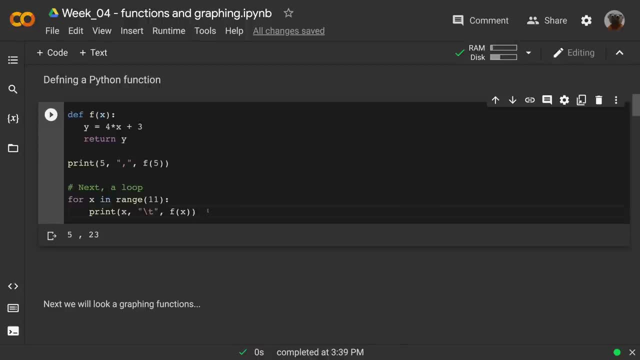 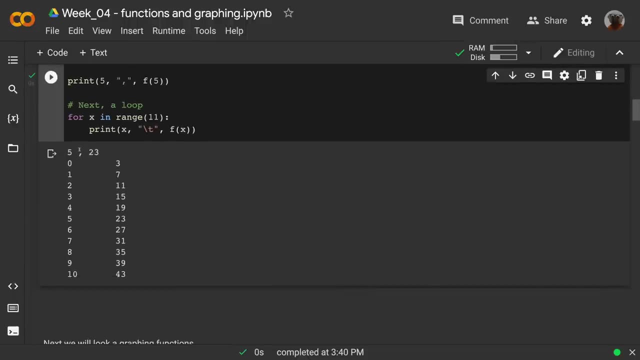 since I defined that function x, f of x, and I don't have my headings here, but I think we can use our imaginations- There we go. So printed that one value, but then in the loop just went through and looped. 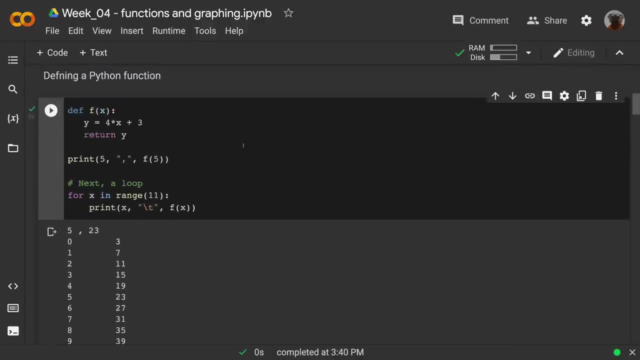 So these are the ways that we can illustrate a function in code And you know what we can do with these functions. you know is almost limitless. You know you can have a function do anything And you can name it anything more. 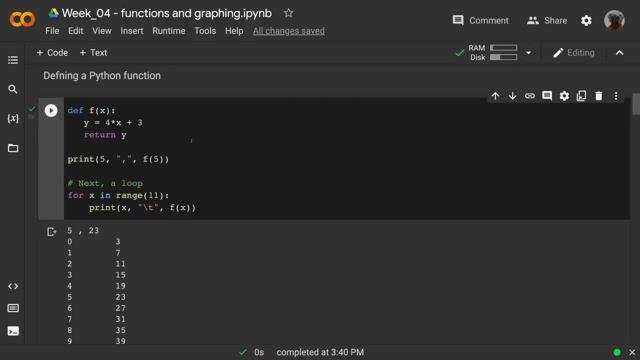 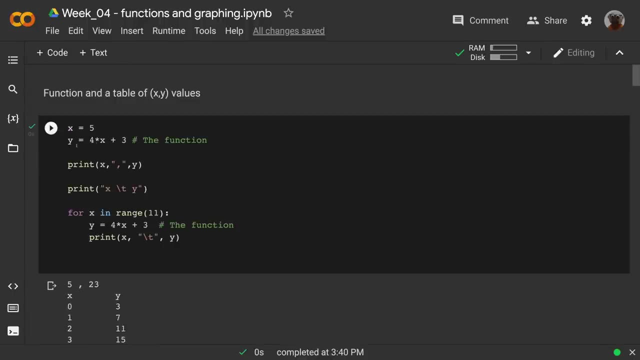 complex than this. you know, give it a word. But I wanted to show you the connection with the classic math notation and functions in Python, Whether I actually just call it y equals- that still works as a function, or whether I define it. And next, 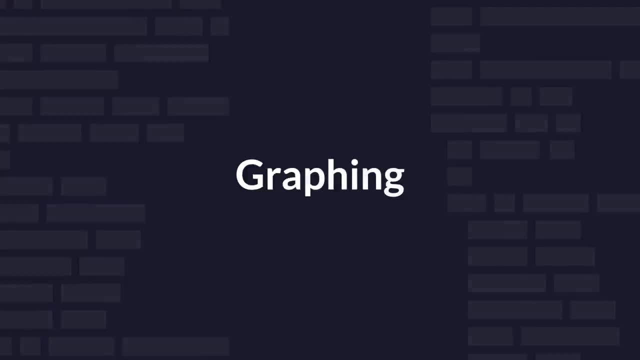 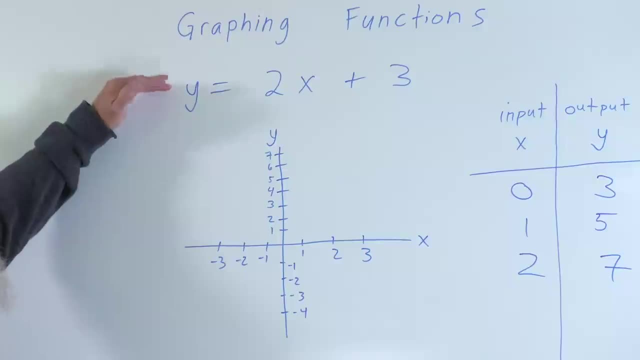 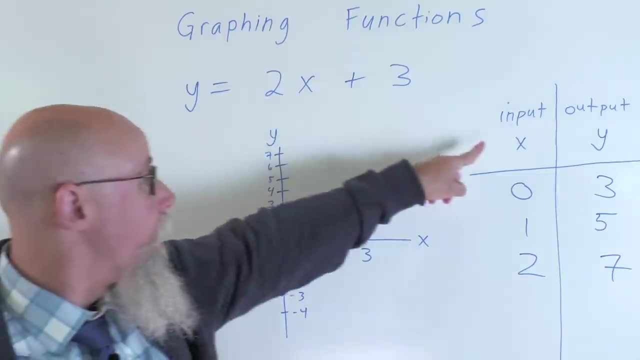 we're going to look at graphing functions. So now, when we talk about graphing functions, we'll use this equation: y equals 2x plus 3, and I'll use the x and y notation. So we have our 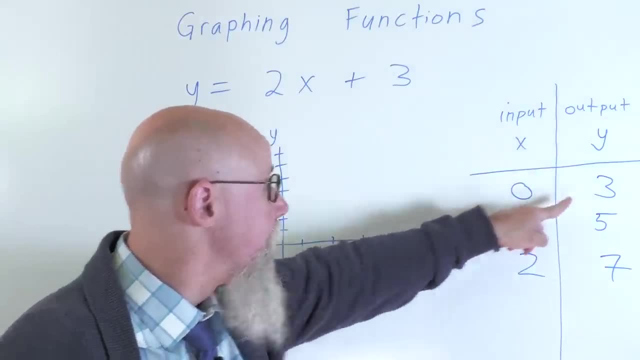 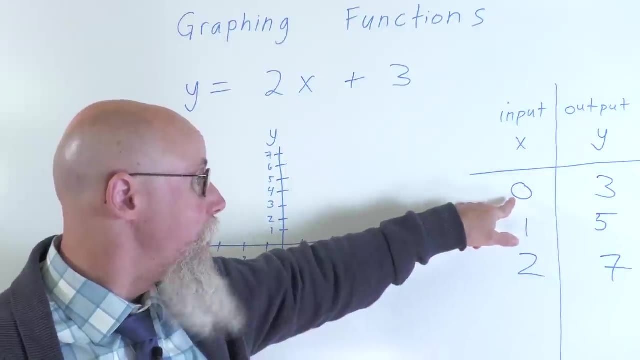 input and output. you know all the different x values and what y values match up. So if you ever come across something like this, you can see that if I plug in both of these x and y, that should make the statement true, And so. 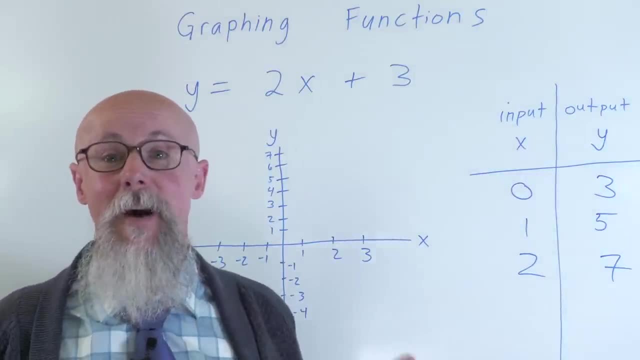 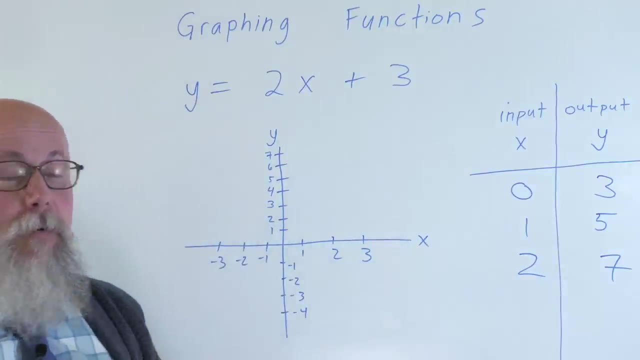 we have a few of our points here And then now we're going to see how that matches up with the Cartesian plane, or x-y coordinate plane. Cartesian, because Rene Descartes invented this. So we have 0,, 0 at the center. 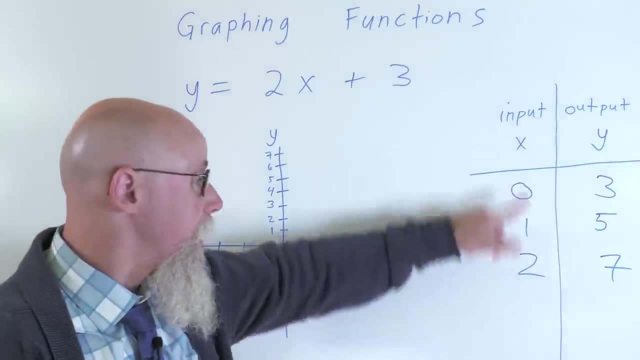 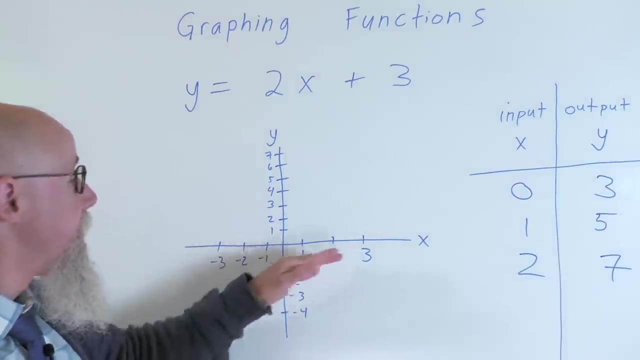 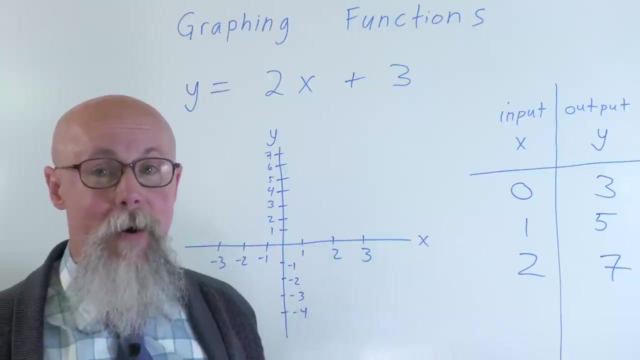 and how much I count for x- positive to the right, negative to the left- and it comes first, like x comes first in the alphabet. Then my y value- positive up, negative down- and my coordinate pair would be my x-y. 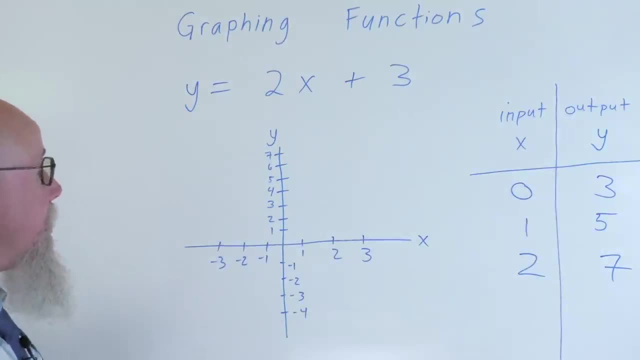 So this 0, 3 would be 0, so I'm not going left or right at all up to 3, plot the point Now. I don't also need to write this, but I'll show you. So then that would be the. 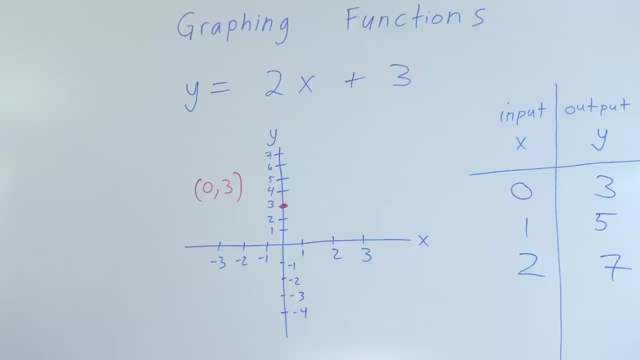 point 0, 3.. So x-y And then 1, 5.. So I would go over 1, up 5, plot the point And then that's 1, 5.. 2, 7.. 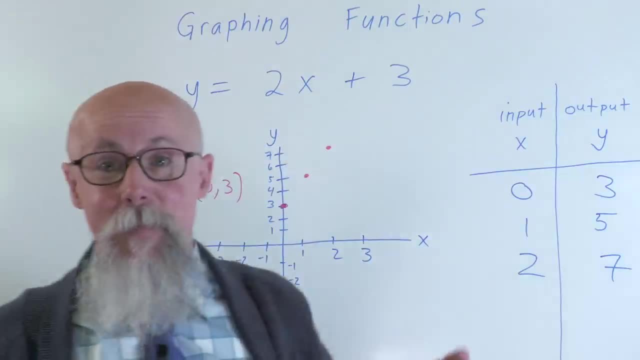 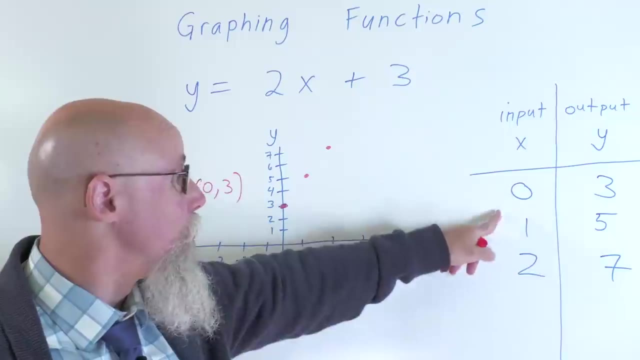 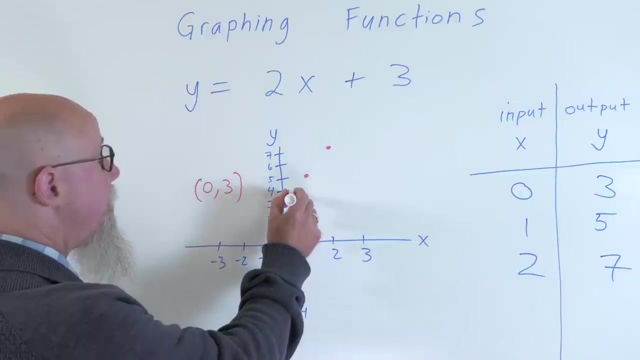 Plot the point Now. I just plotted 3 points, but I'll tell you, if you really wanted to try many in-between points- decimals or other numbers that are in-between- you could bet that each of these, whatever you know- 1 point. 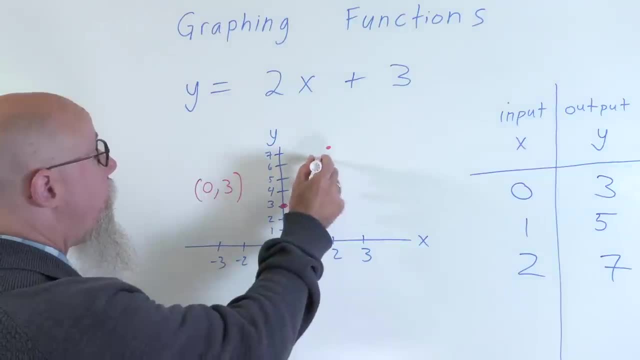 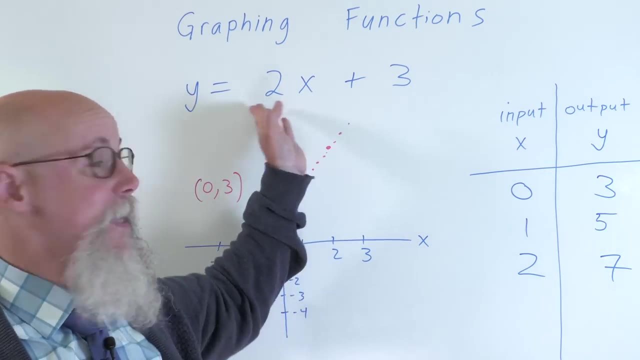 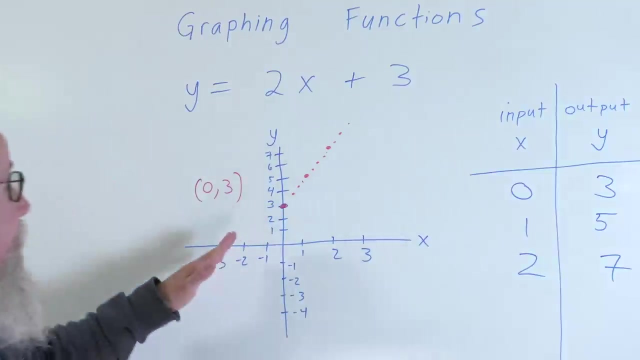 something. 2 point: something they would all end up being on this line: It's continuous. There's no x-value that can't go into this. Whatever weird fraction or decimal, you know, mixed number, anything, So all the numbers would. 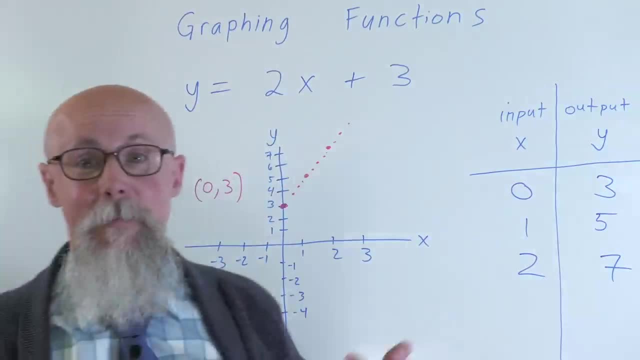 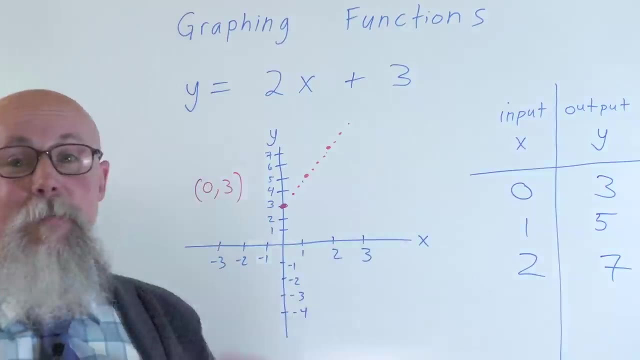 be on this line. So with this type of function, we're going to call it linear and we'll get into other types of functions. But that's where we plot a few points and then we want to look at these patterns. 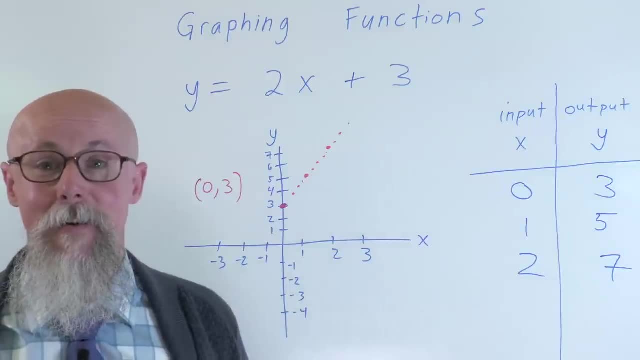 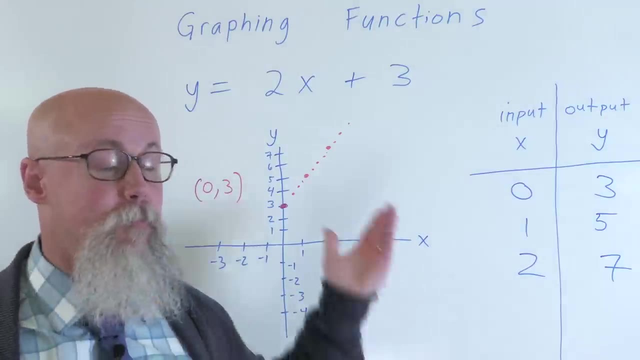 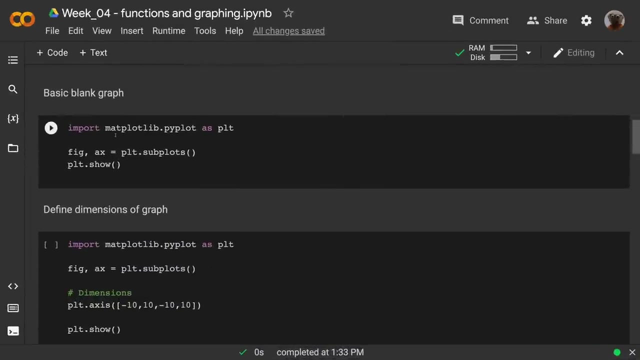 What type of graph does this end up looking like? So what we're going to do now is look at in the Python code how to create a graph and plot points To make a basic blank graph. we're going to import this library, matplot. 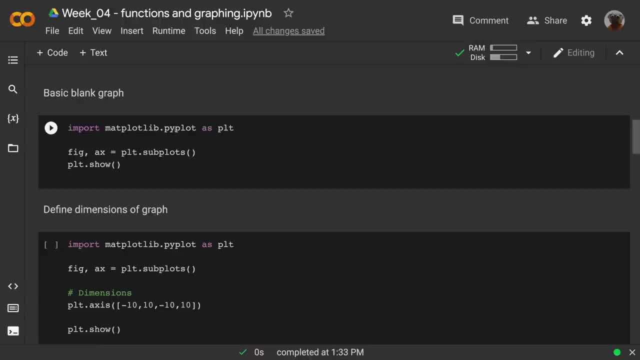 lib, pyplot, and that's a lot. so we can import this as plt, So I can reference this whole library as plt from here on out. And here's what we're going to do. The first line is, these are: 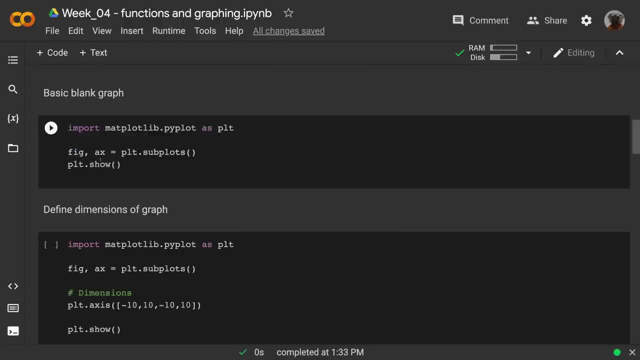 standard variables that we use: fig for the figure, ax for the axis. So these two variables and that equals pltsubplots. And then that sets this up and we'll do pltshow. There you go: Import, set this up and then show. 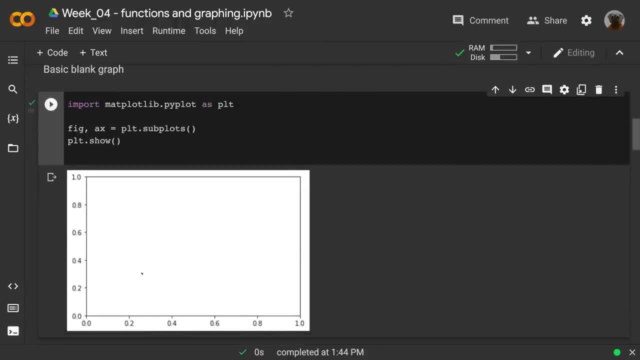 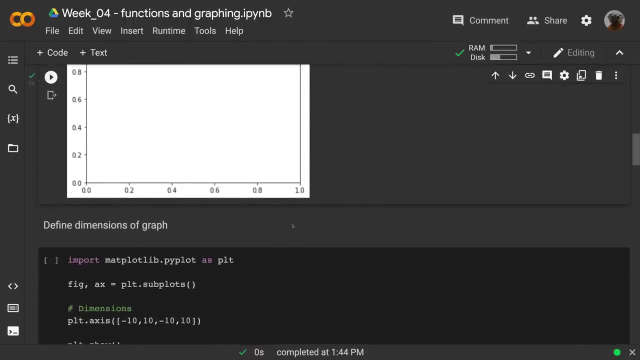 And then that gives a basic graph. These are all the defaults, nothing else going on there. And you know we have this set up, So we're going to build upon that. Now let's define the dimensions here. Notice, that was all just the first quadrant. 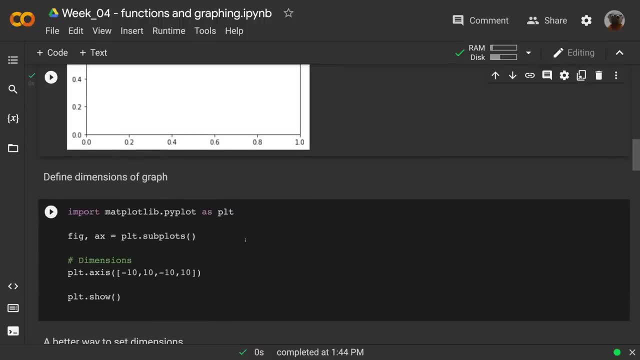 everything's positive and even only goes up to one. So again, import, matplot, library, pyplot. We set that same two first lines, but now let's take a look at these dimensions. Now I have that plt. 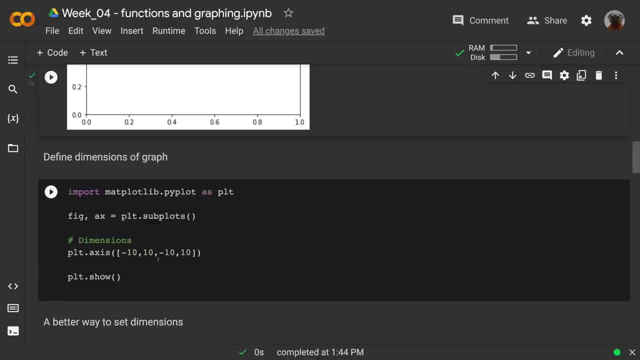 so it's pltaxis and I'm going to set this axis Alright, and it gives you the range of x values and y values. I'm going to show a better way in a second, but you can do this on one line. Here's the dimensions. 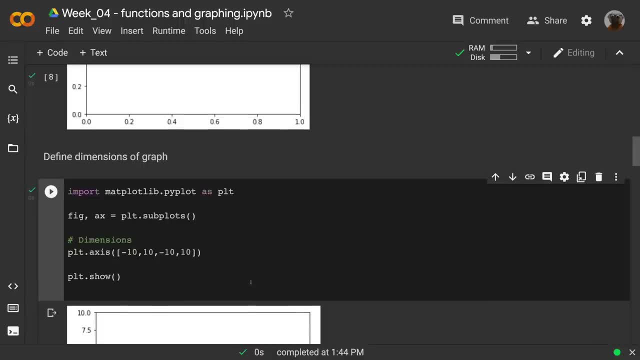 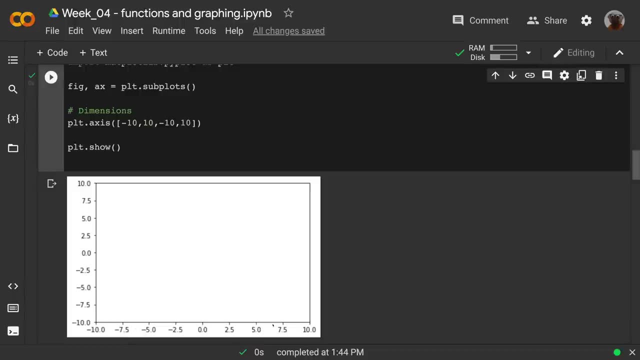 and now, when we show it, I want it to go from negative 10,. we see across the bottom, the x-axis, negative 10, up to 10,, 0 in the middle and on the y-axis, negative 10, up to 10,. 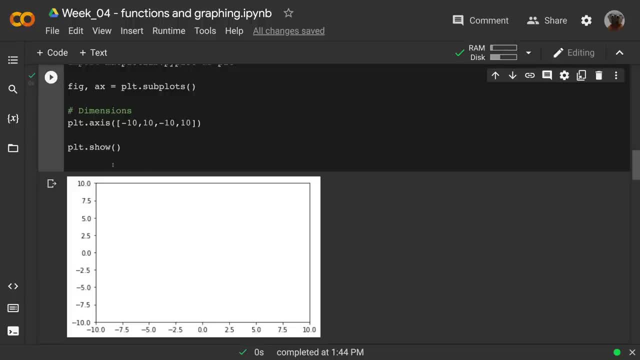 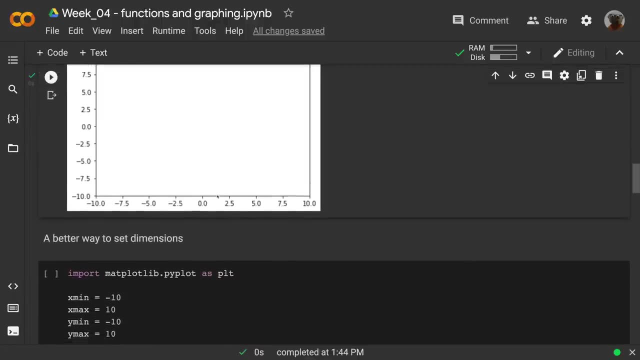 0 in the middle. That's great, but I have no lines, I have no axis and, you know, not the clearest. So first of all, here's a better way to set the dimensions. I'll define them. 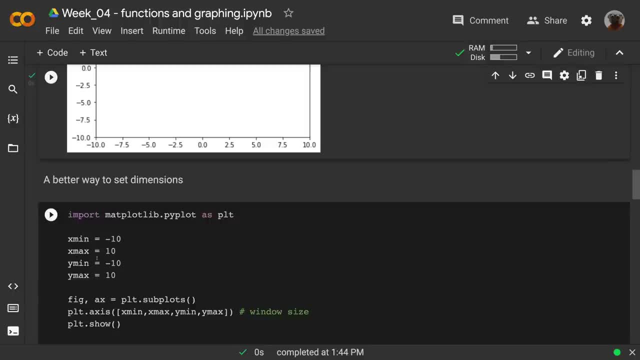 right at the beginning, as variables: xmin, xmax, ymin, ymax and that way. alright, I want it 10 in every direction, and I can set them here, Easy to see it, and change it if I want to. and now, when I do all this, 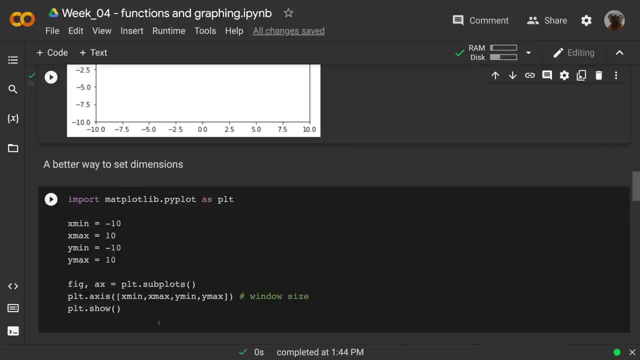 this is really what I'm doing when I set the axis size: xmin, xmax, ymin, ymax. That's really the argument that it's taking, and it becomes a lot clearer when we set it up like this. So then I have this. 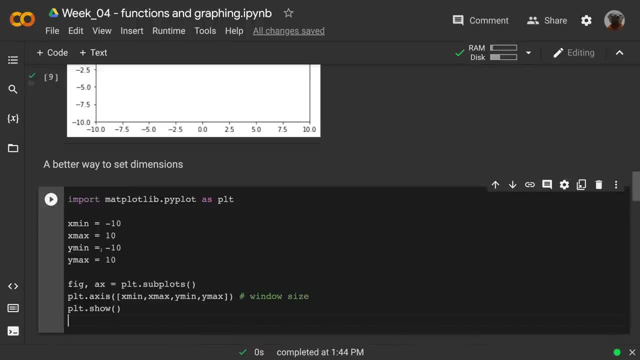 and I can set this and then, if I wanted to, I'd say, oh, for this one. this y value goes really a lot higher, so maybe I want that y maximum to be 20 instead of 10.. And then when I run it, 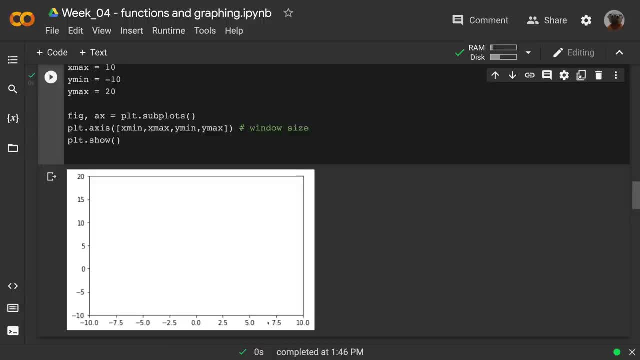 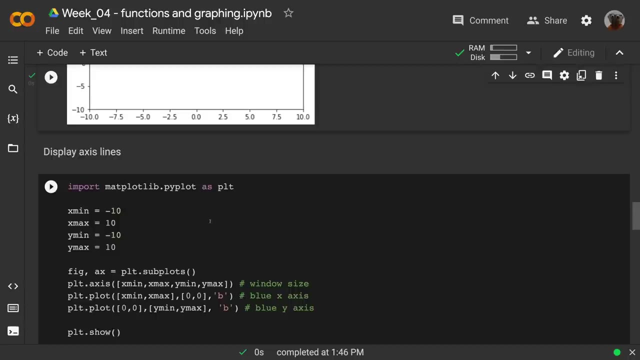 now notice the size of this still looks the same, but it adjusted accordingly. and on my y-axis it goes up to 20. And on my x-axis, negative 10 to 10.. So let's display axis lines here. 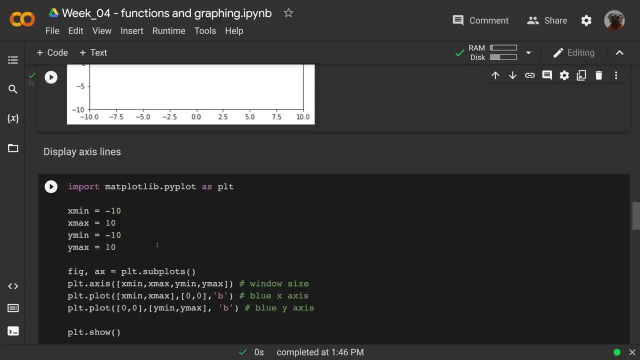 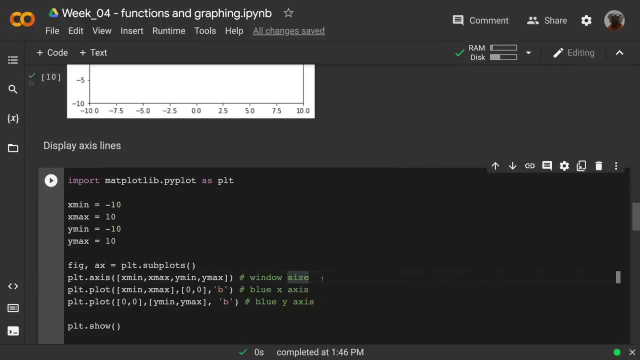 If I have my dimensions defined, and now when I plot the axis, well, that's the one we already did here- the window size, but I'm going to just plot them as lines. So this line, here I have xmin. 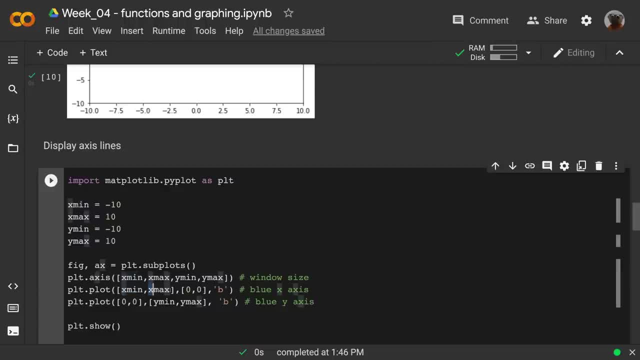 xmax as my array of x values. See notice, it's pltplot and I have my array of x values and then my array of y values And the default is to make this a line so it won't just plot two x values. 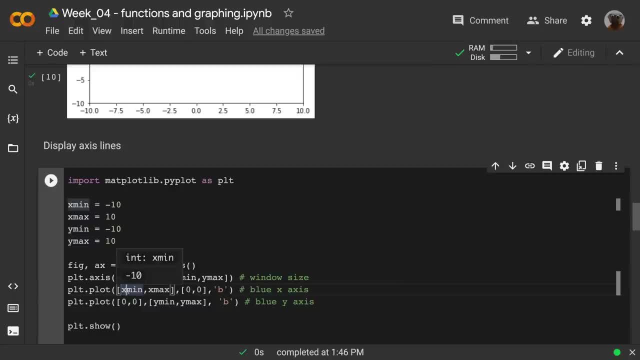 and two y values. it'll draw the line from xmin 0 to xmax 0, and this b in quotes makes it blue. So we're going to do the same thing with the y pltplot and my x values are going to be 0. 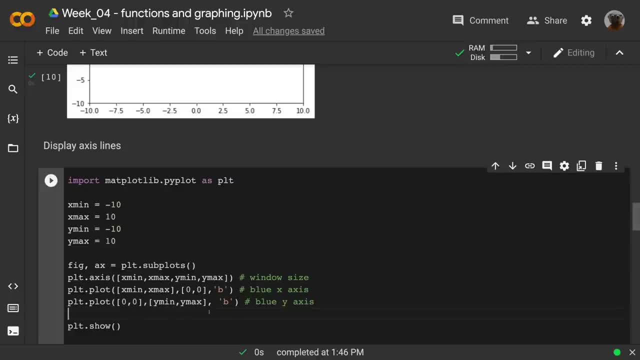 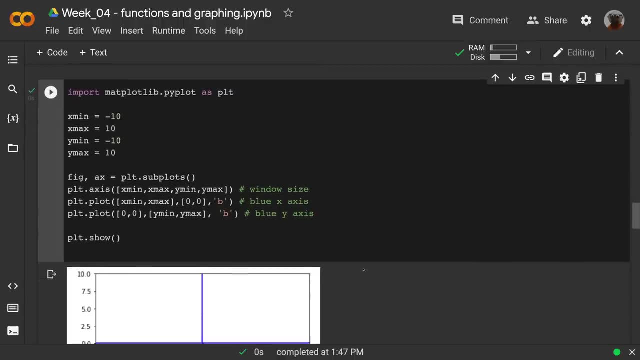 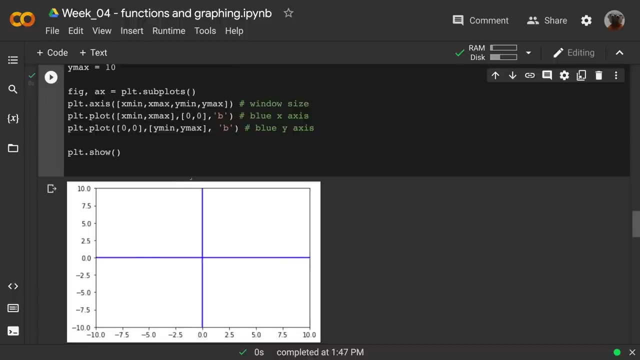 at 0, ymin, 0, ymax, and then I'm going to make that a blue y-axis, Just because I like blue, And there we go. So now we have this, that will give us our xy-axis. So, from everything. 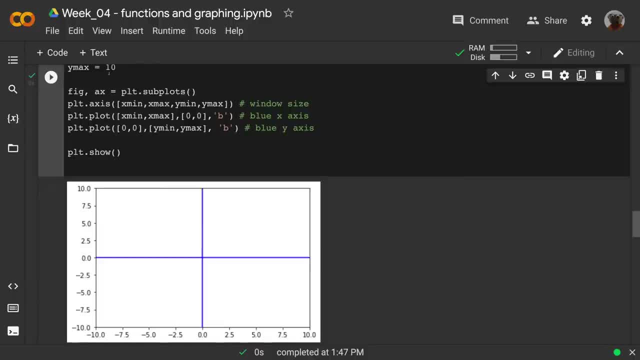 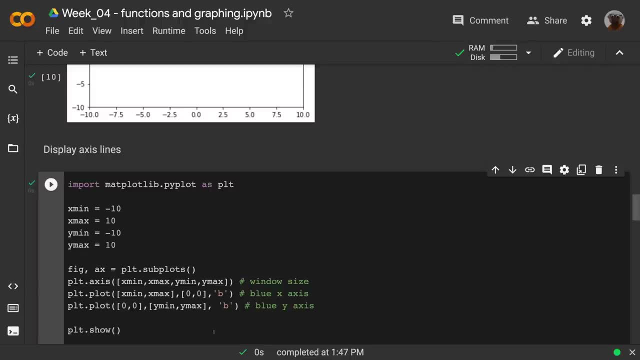 we do now. we have an axis, we have a point of reference, So everything that we plot is going to start with this. now Define the dimensions, set all this up. we might not even need to change any of this, and that's going to give us. 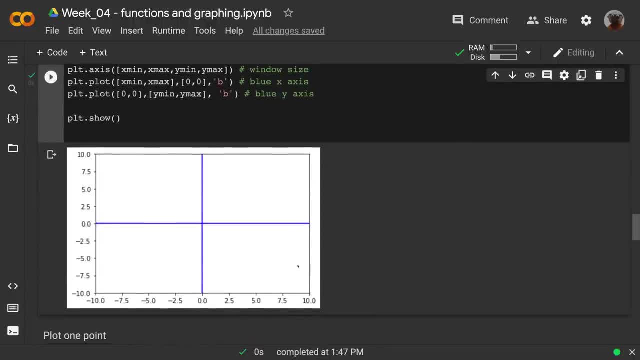 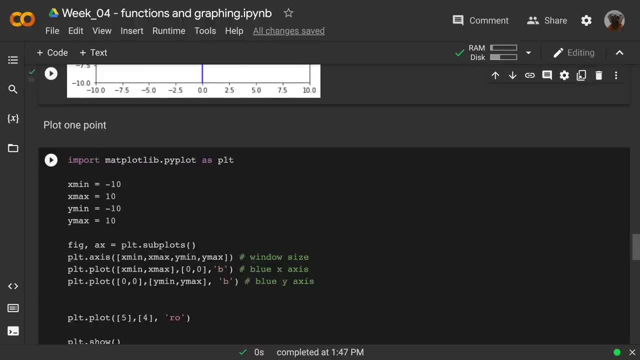 our graph with an xy-axis. Alright, so how do we plot one point? So we see the axis, the default is a line and I made it blue b in quotes. so how do I plot a point? Well, I make. 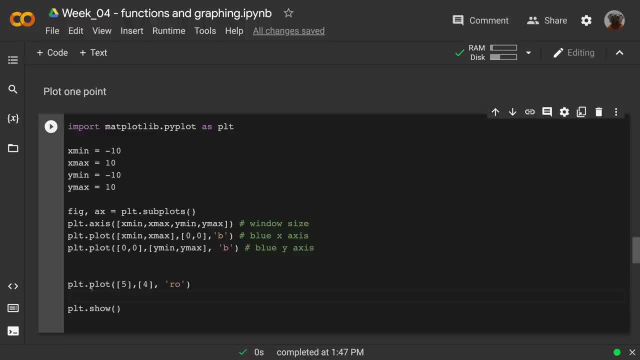 this line. here I have an array of one value, which is 5, for the x value, one value which is 4, for the y value, and then the r makes it red and the 0 makes it a circle. 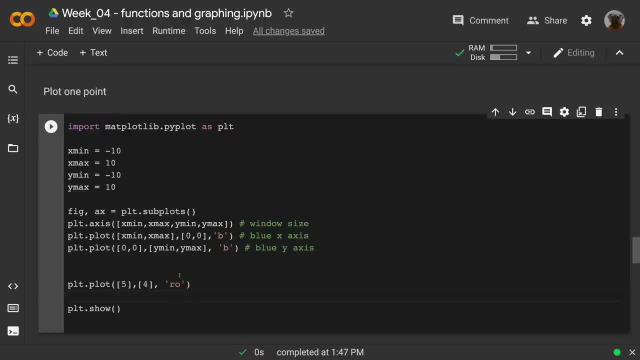 Actually, that's o. So there's some other options you can do. You can do a dash, you can do different symbols, but for right now I'm going to make this a red circle And that's how we make that here. if I have these two, 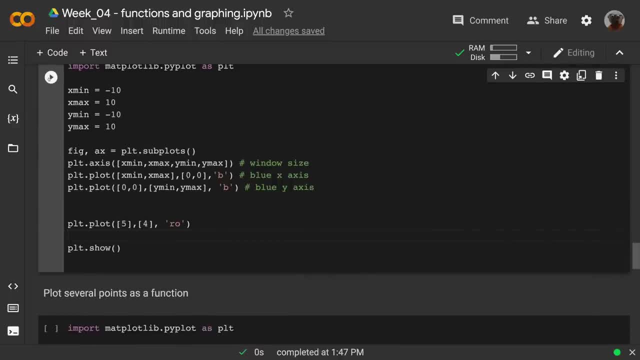 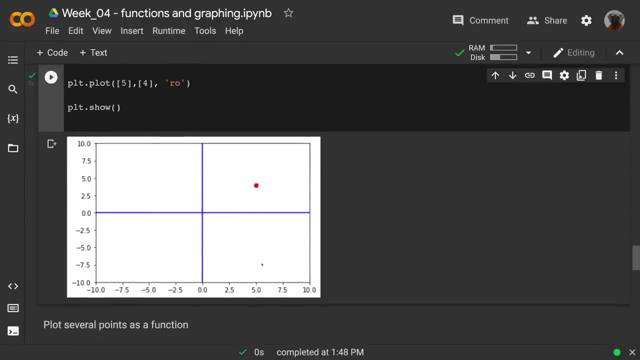 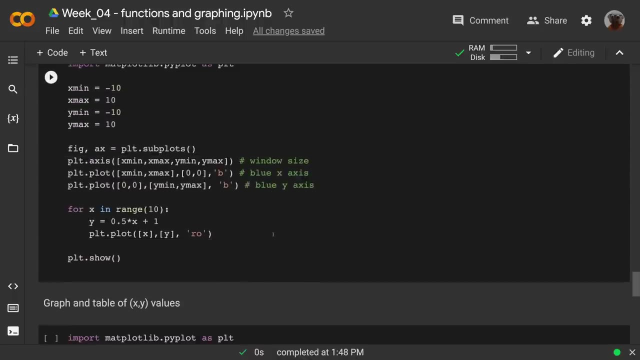 And so when I run this, it'll still plot those as an axis, and then we'll do 5,, 4, and then that's going to be a red dot. Alright, so if I wanted to plot multiple now connecting with what we were, 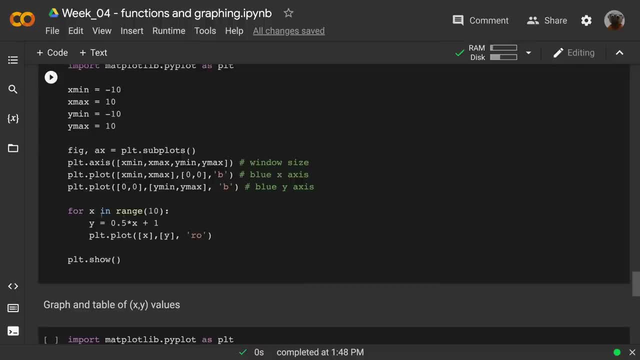 doing with the functions. here I'm going to set up my graph and here in my range I'm going to have the range from 10, so I'm going to go from this, from this value, my y value. 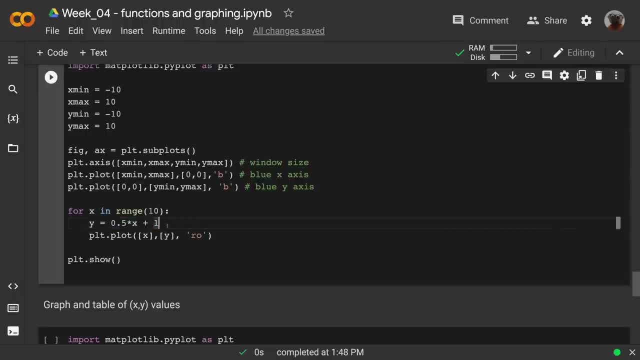 y equals .5x plus 1.. And in this case, instead of making it a table, I'm going to plot pltplot and I'm going to plot that xy value as a dot. So this range, and I'm going to plot these. 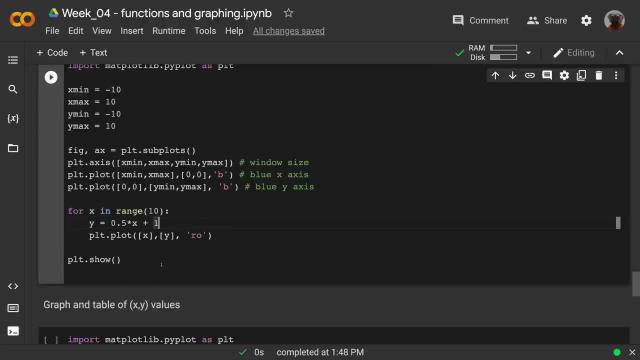 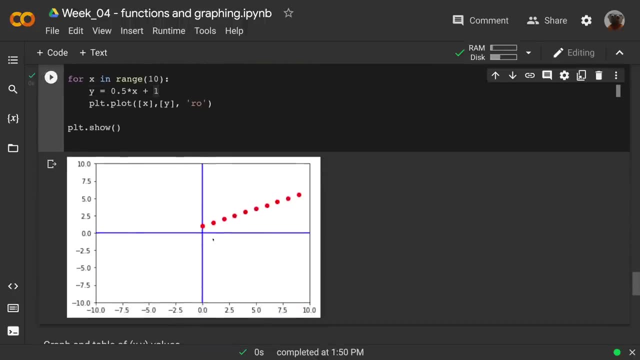 xy values. and again, that's the essence of graphing a function. I have all these different values and when I plot all these points I'm going to see this nice pattern emerge, that this all lines up, And I'll tell you if I plotted. 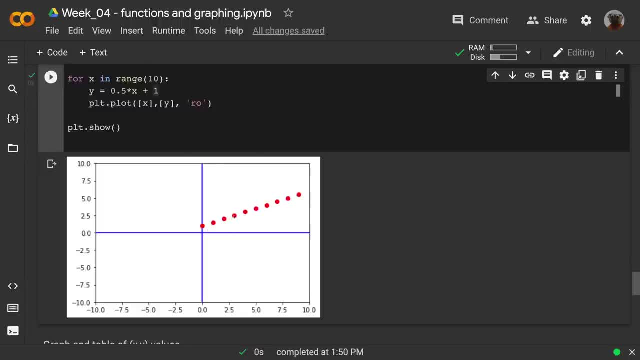 points that were in between. whatever x values there would be, they would also line up. That's why it's a linear function. The graph of it's going to be a straight line And then every point on this line, every xy value. if I plug in this, 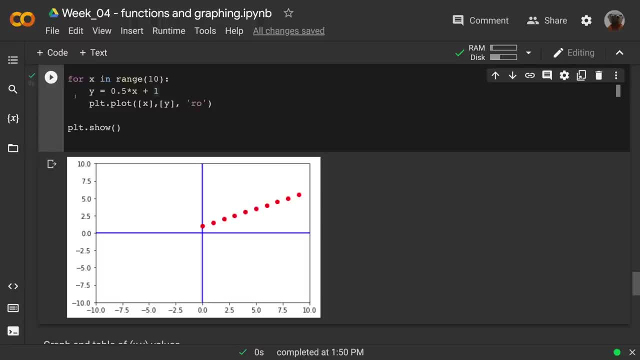 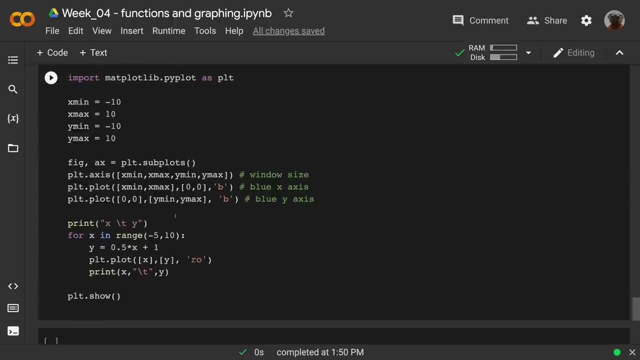 function. it's going to work. So my loop to graph a function And here then we'll create a loop to do the function and the table. So, like we were doing before, I'm going to build upon this basic graph that I have. I'm going to 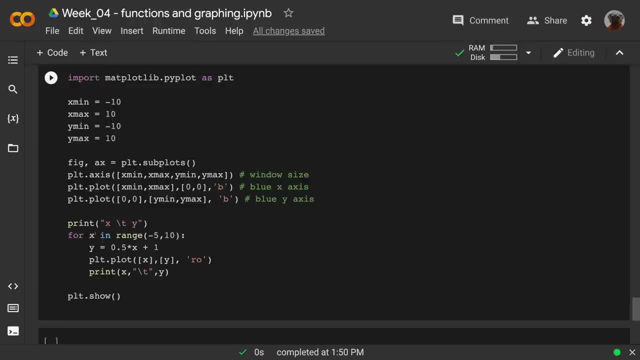 print the x tab y for the heading of the table And then in my loop I'll use the same function here. I'm going to plot the point and I'm going to add it to the table And all these. it actually won't plot all the it'll kind of. 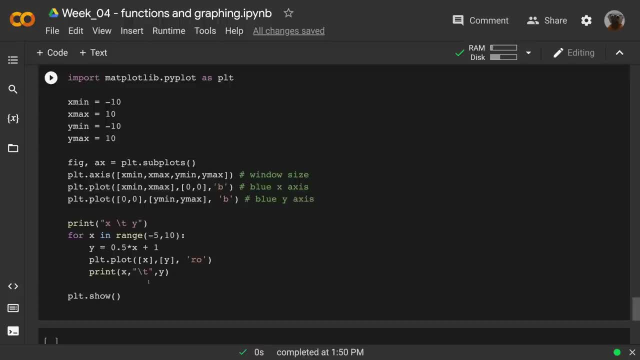 save these points And it won't plot them all. It's really just going to add them all to the table and display the table, because it really doesn't show the graph until the last thing outside the loop here is going to be pltshow. 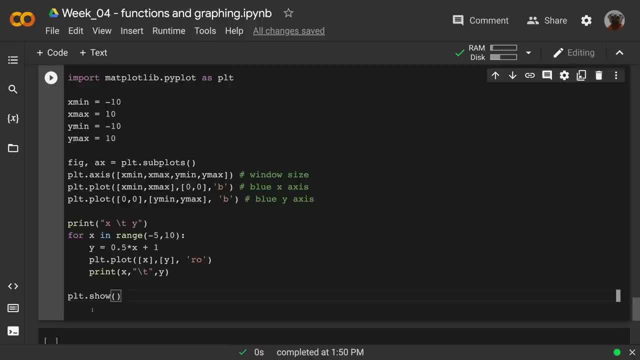 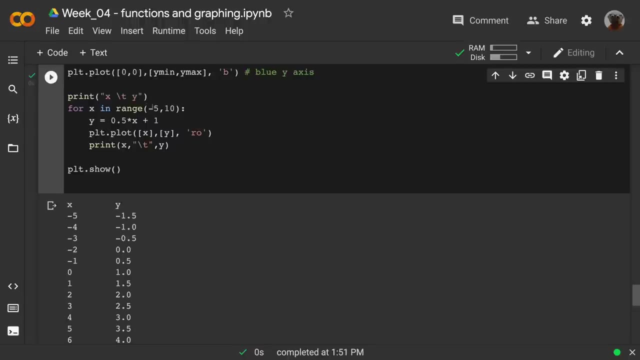 When you have graphs. I think Python just likes to have that pltshow last, So do your other stuff first and then show the graph. So then we have this and we have our table of y values. Notice if I just put one number in the range. 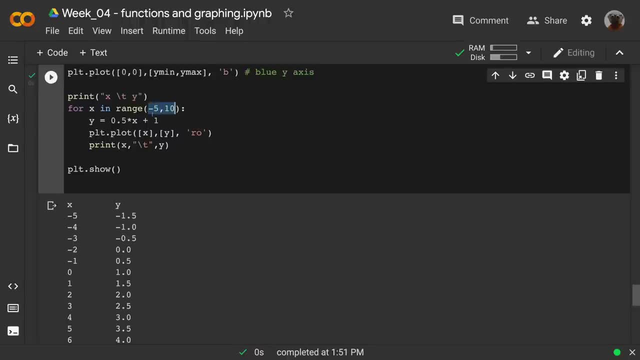 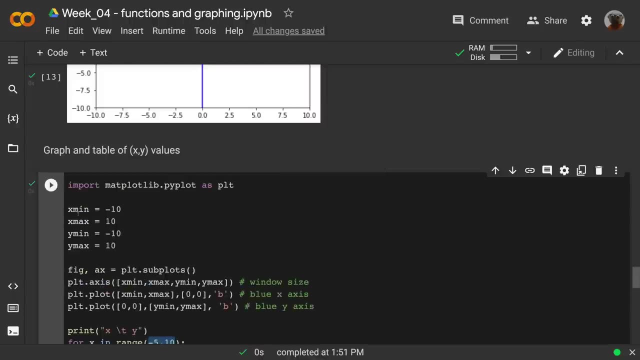 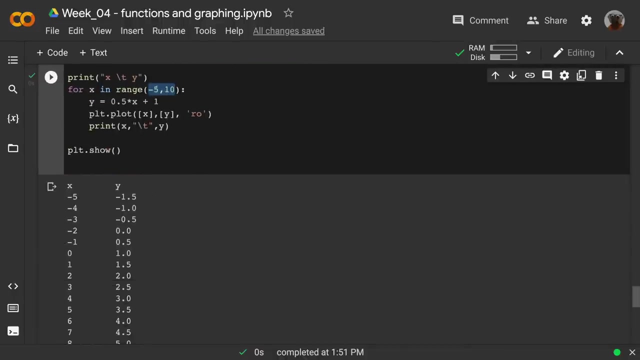 it'll do zero to that number. but I can have negative five comma ten, or I could even just go back to those original values that I defined up here and make this x min, x max, You see, And then you can put any two numbers in here. 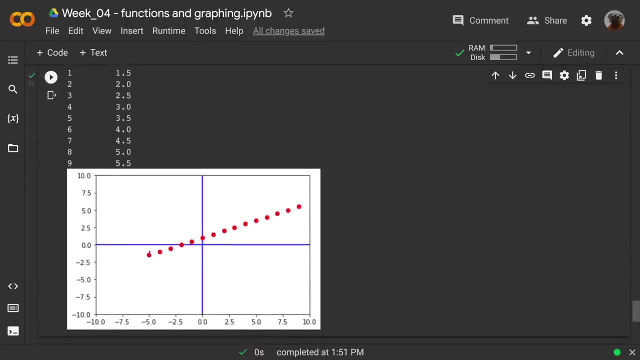 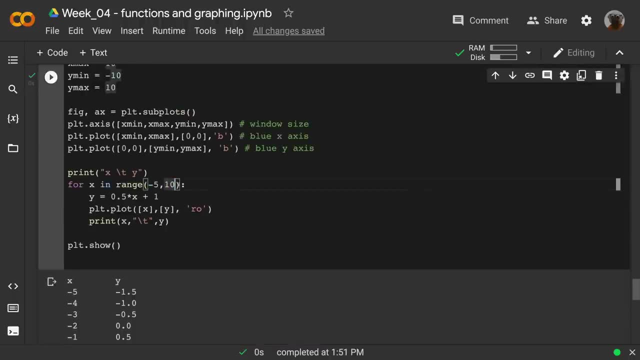 and it'll do the range between there. And you see, it just abruptly starts here and abruptly ends here. But I could change that to make this x min and I can make this x max. But remember, I want to graph that last point, so I'll do. 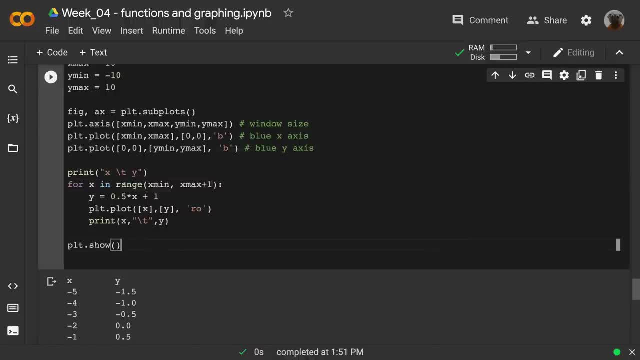 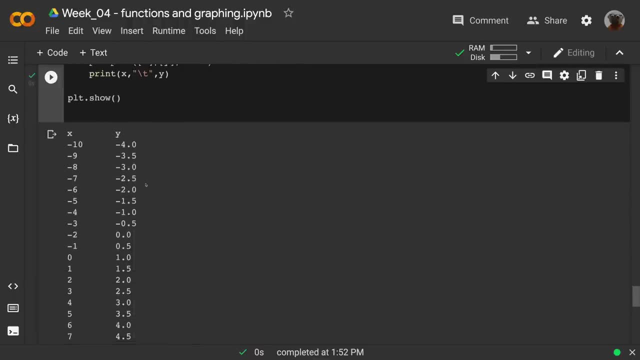 x max plus one, And I can have that range. And now it'll give the full table of values And it'll graph the full dimensions. So there we go. We see what we can do with the function. I have, whatever. 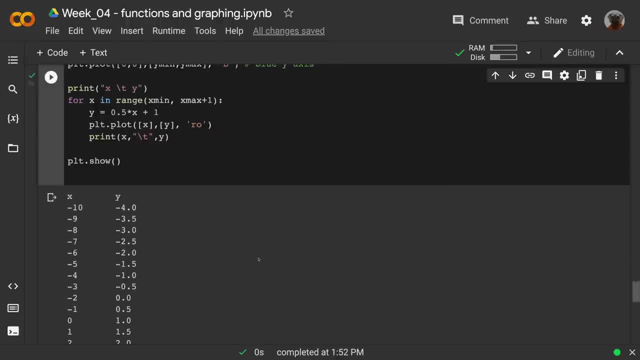 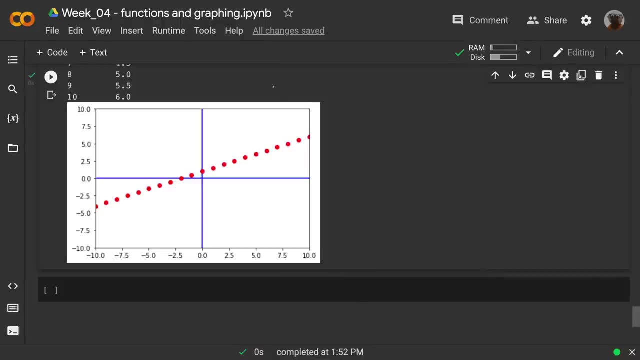 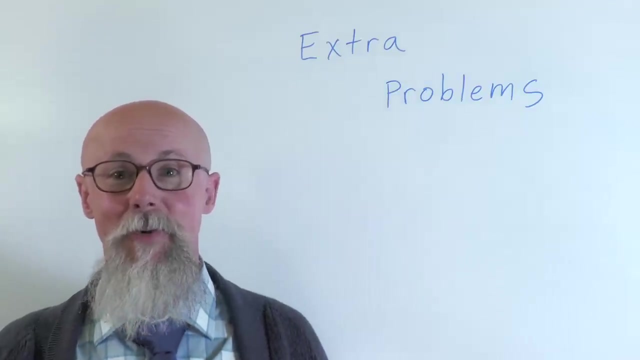 math function. I have plug in different values and see the results, See the numerical output, see the graphing output and now we see the connection of graph, the table and the functions, Now that we've worked through the core skills in this unit. 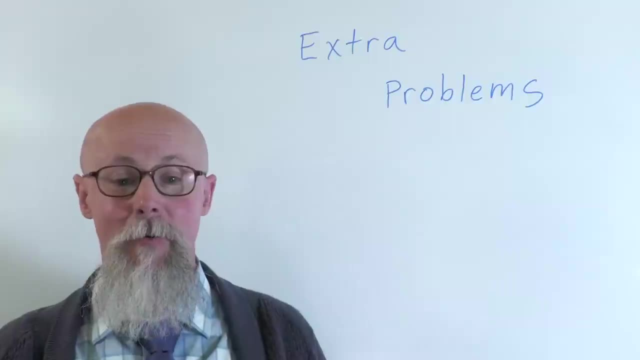 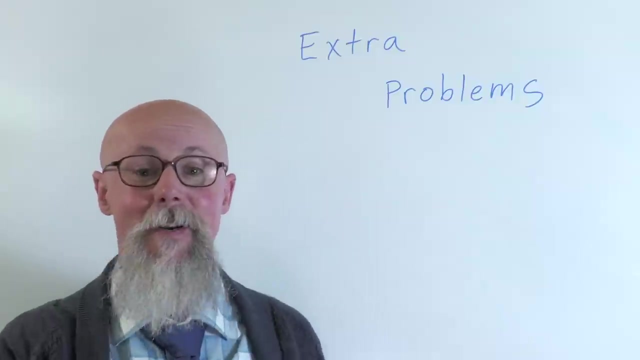 let's look through some extra problems, and I'm going to work through extra problems using the Colab notebook, So you can see how you can apply these resources that you're building and use these to solve problems that might come up in a textbook or 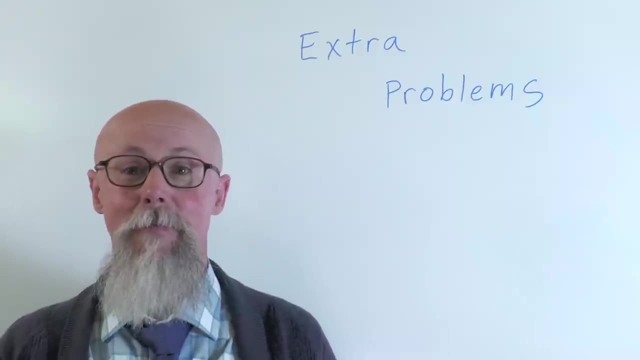 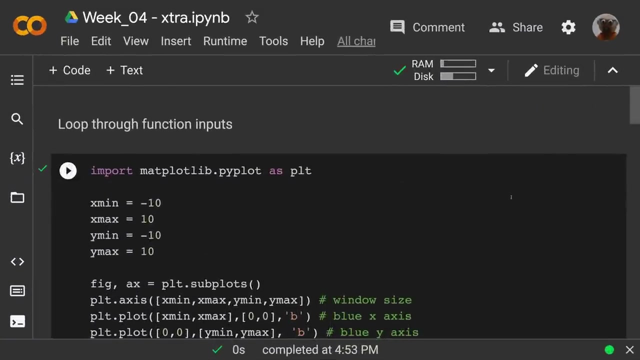 in day-to-day life. So we're going to go through some more extra problems here. So let's talk about more ways to graph and more things we can do with the graph, Because we want to be able to display our data, our 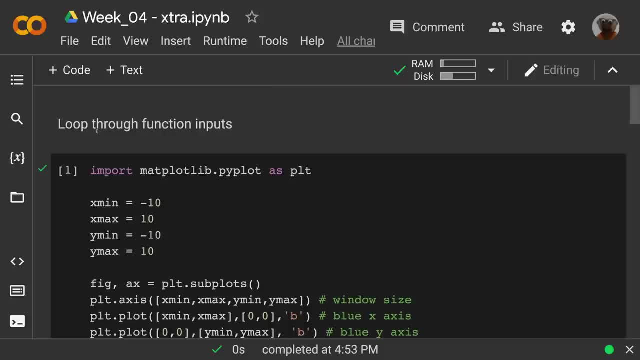 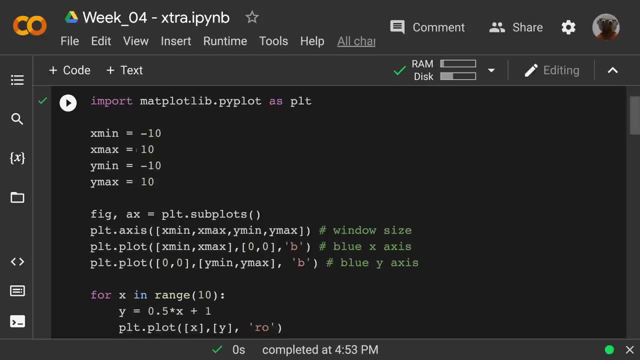 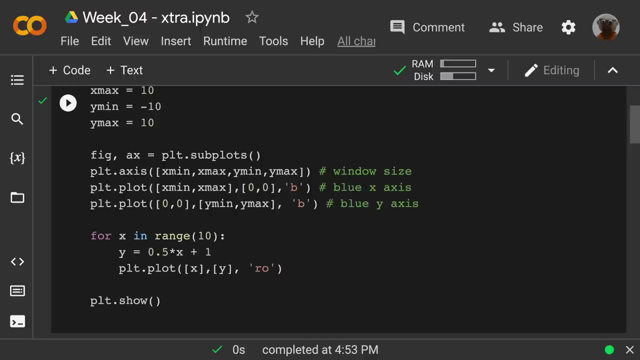 functions. So we did look already at how we can loop through inputs. I can define my graph and we already did this: The x min and max, y min and max. and we talked about how we can loop through. I get x in a. 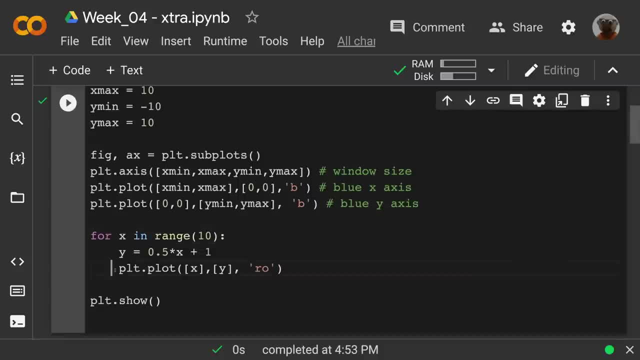 range and then each time I'm going to plug this in and plot that value, And that's the idea of the function: That each time I get an x value in this range, plug it in for y. plug it in here, get y. 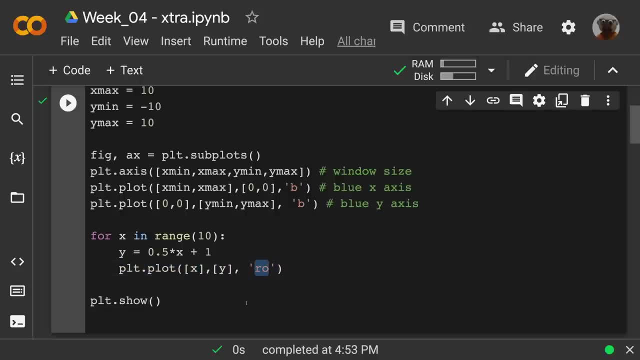 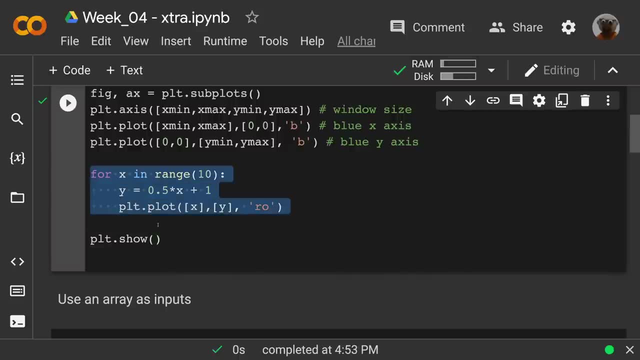 and I plot that xy point, In this case as a red dot. After doing all that, then we show the graph. But what if we didn't have to do a loop for our input? What if we could use an array and 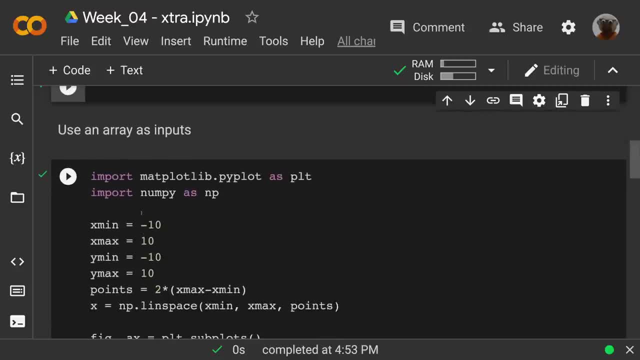 we'll revisit this again in other units, but we have this numpy array and it's not that long of a word, but it just seems to be the convention that we imported as np, And so you'll see a lot of examples throughout the 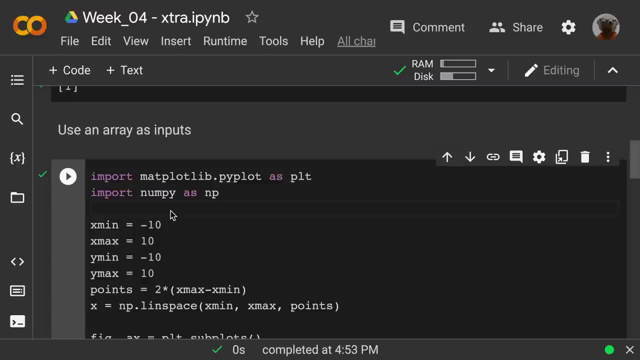 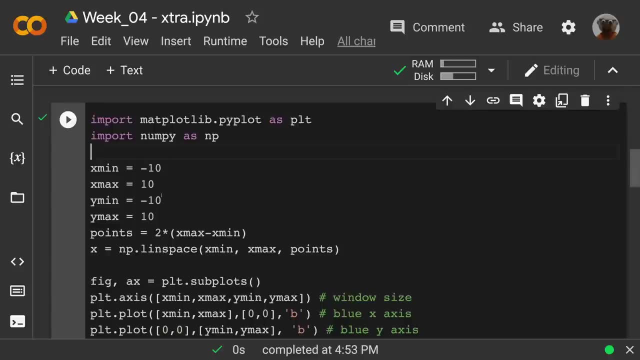 internet, that np dot this or that. So that's what we're going to do. And again, defining x min, x max. So, given this numpy array, here's what we're going to do. Then, given these values, I'm going to define how. 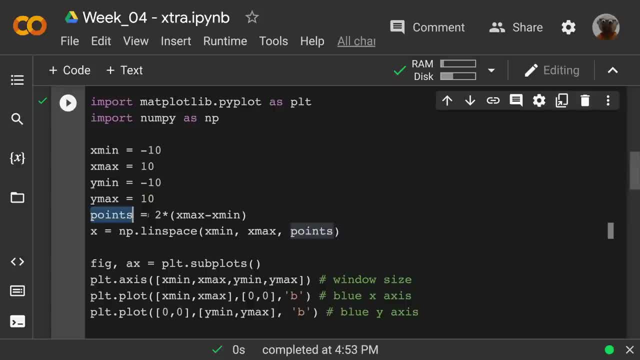 many points I want in my array And in this case it's going to be 2 times x min. max minus x min. I feel like that's probably enough for our purposes. but that number 2, you can up that to 10 or whatever. 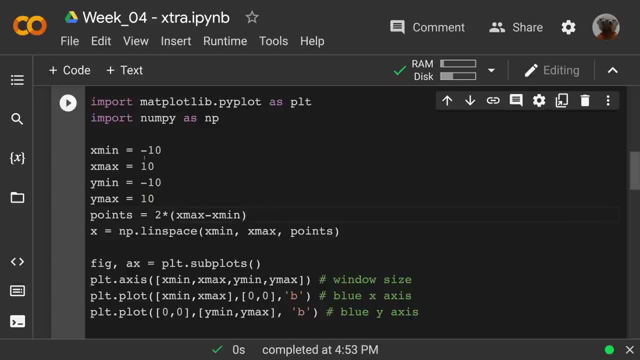 you want, And then we see. so then we want to make as many things dependent on these values as we can. That way, if that changes, if I change my window, everything else will change accordingly And I don't have to go through and find all these. 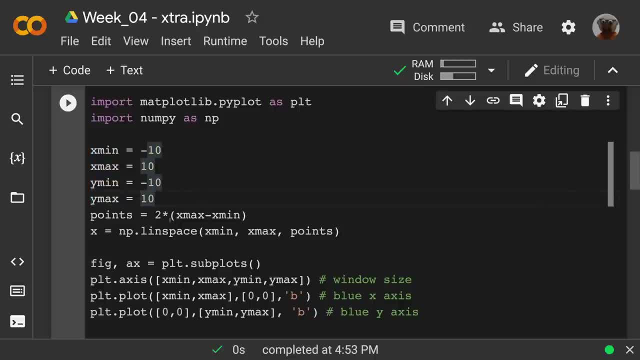 variables. So, yeah, I get the full range times 2, so that's 2 points through. You'll see that that's actually going to work out just fine, But you can always increase that. So now that I have any points, this is how I define my. 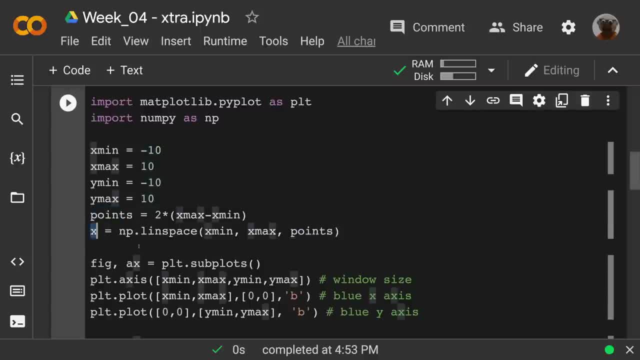 array of x values, And since I really am only using this once, I'm going to just call it x, because that is my array of x values. And so, numpy, we have nplinspace, So we have this function here which is going to set up our array. 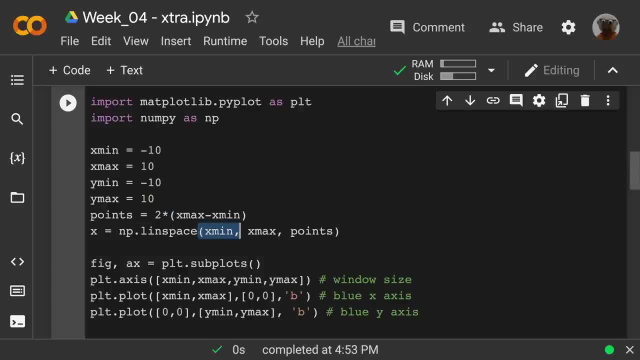 You know space for linear graphing. So it takes the argument: where do I start, where do I end and how many points do I have? So we see, we just make all this dependent and then I get my x value. So this: 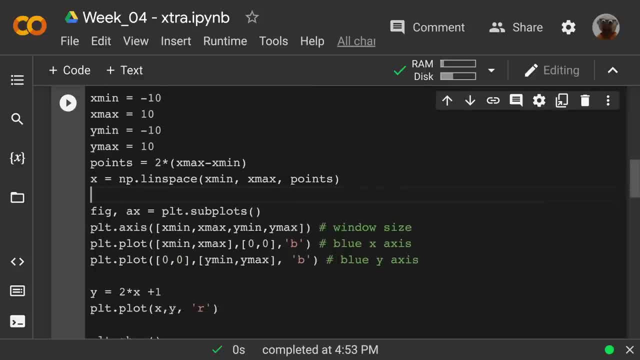 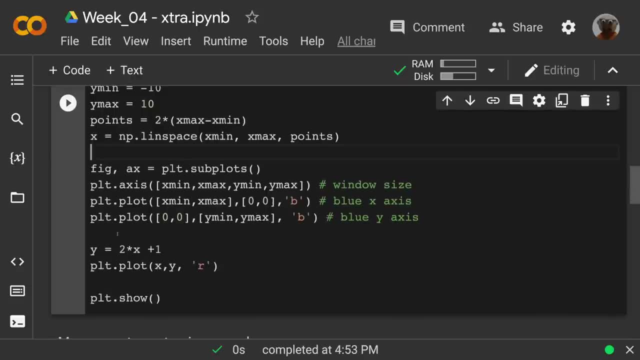 saves us the time of having to do a loop. Python will do this for us. Here's all the graphs, and we're going to talk about how to change some of this stuff too, in a minute. So now I'll just I like to define my x value up there. 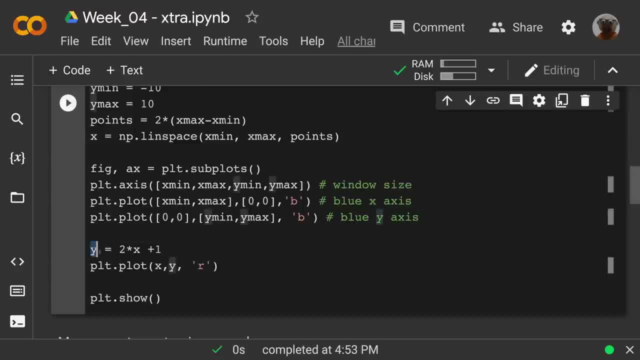 right where I have number of points in the range. So I have my y value and for our purposes here we'll just call it y equals. but you can graph multiple things on the same axis and you can have it y1,, y2, whatever you'd like. So 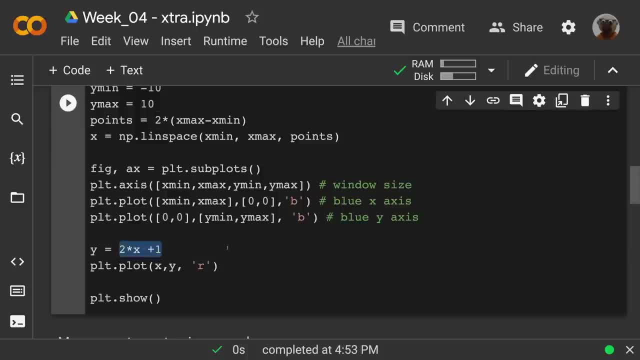 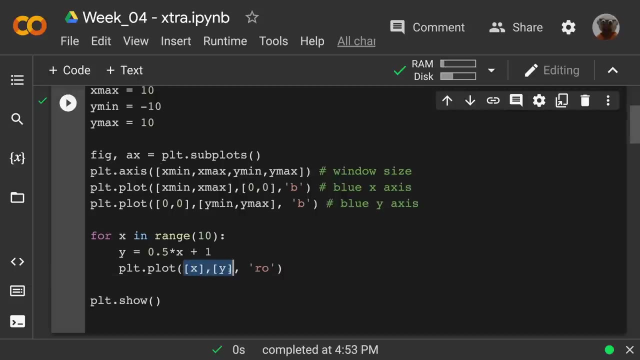 I just defined this relatively simple linear function here. So then, when I plot, I'll plot x and y, And if you remember, before we were plotting x and y each as an array, in this case with only one element, But here 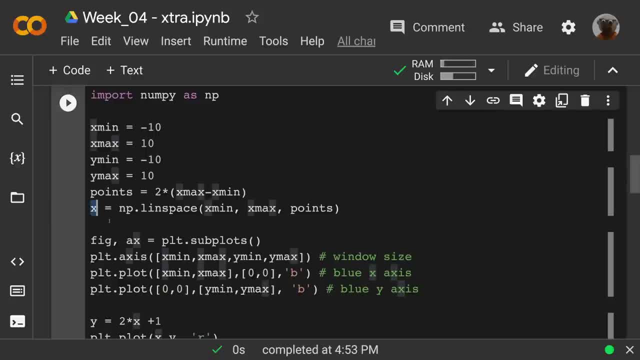 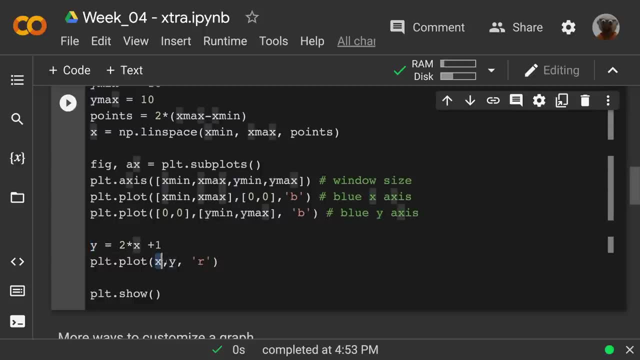 you see, I defined my x value as an array of x values and therefore y becomes an array of y values. So I can just reference these variables- x- y, because they each do represent an array In this case. then I decided to make the 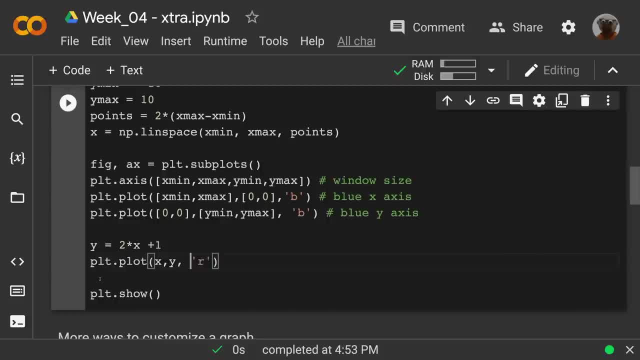 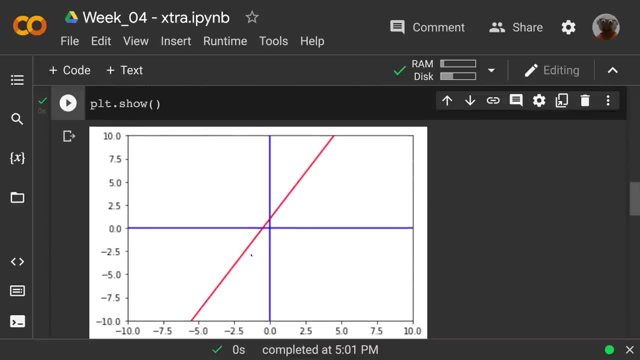 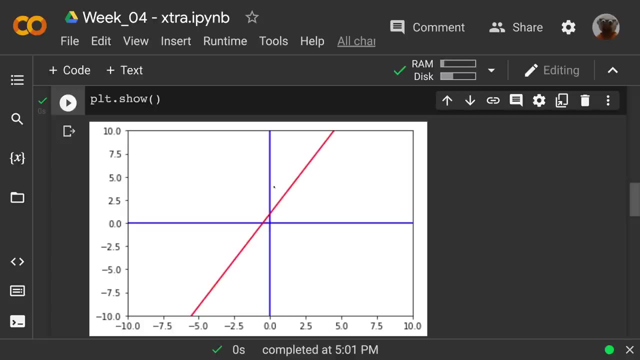 line red. so I put it r in quotes. So there we go, And when we graph this, then we can see. I have my graph and that looks about like that would be 2x plus 1 with the red line. Alright, so let's talk about. 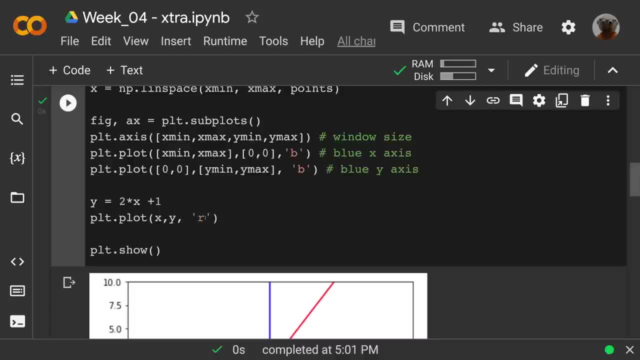 some other things we can customize here Now. yes, r g, b work well. I just had to put b for the blue line, r g for green, and if I want it to be a black line, then I will put k. 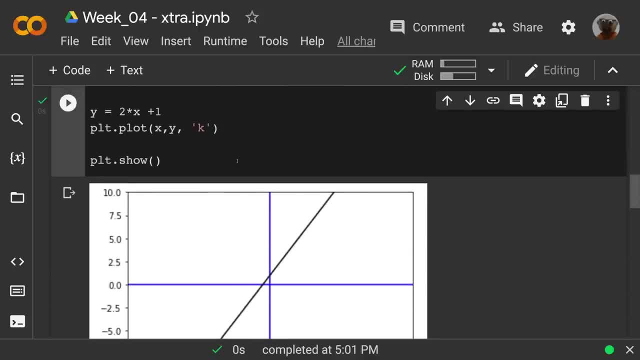 So you see r, g, b, c, m, y, k. those all work as simplified ways to define the color of the line. If you don't put anything, Python will actually assign a color to each line And it'll cycle through, so that if you plot, 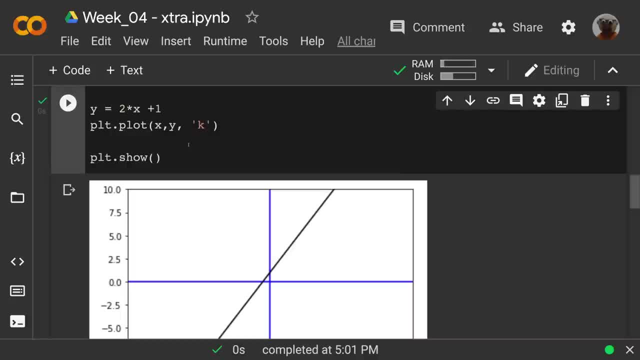 a few lines, they each get a different color. But if you really say you know, I want it specifically to be this line for this color, you can define this And then, other than those major colors, you can actually just write. 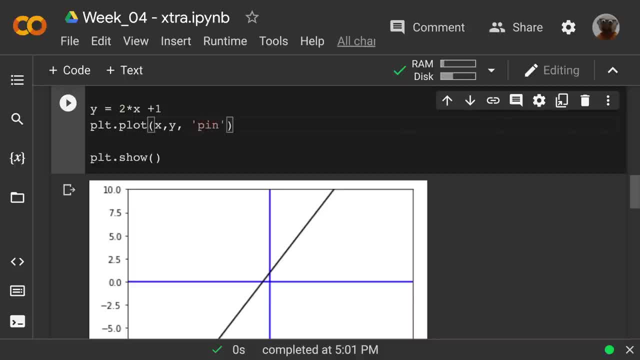 in colors, then it. you know there's no one letter abbreviation for pink, but if I want my line to be pink, I can write in the word And I can't say: like every color that will be acceptable here. but 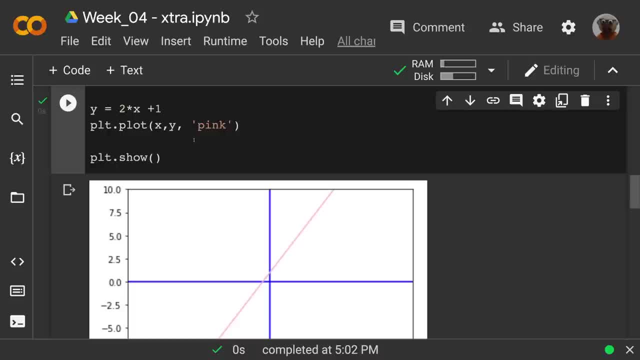 it's gonna be a bunch. you know, If you want a line of a particular color, type it in, try it And there we go. So we have all these different ways to define the color of the line, Because- remember, 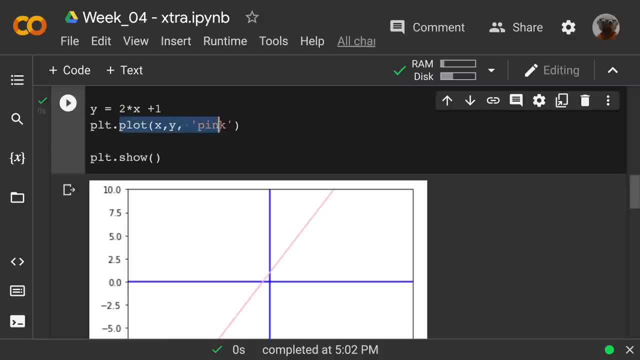 this plot. when this plot graphs, the default is that it's a line. So if I want it to be a point, then I would have to define these definitely not as an array, but, um, as each an array of one value. 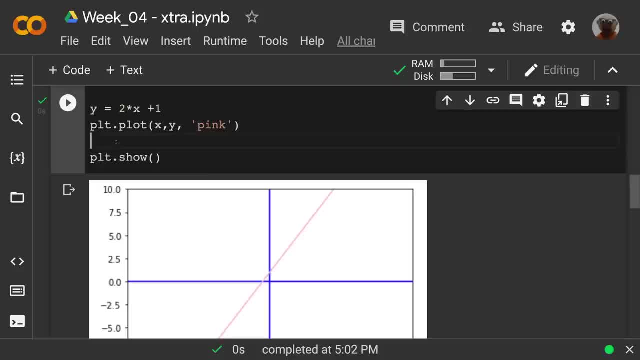 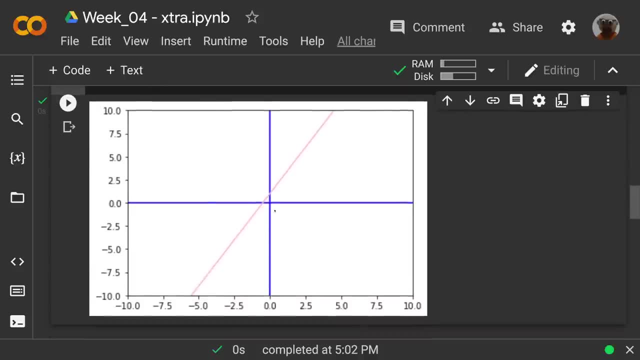 and then the letter, but then something like O for a circle, or the carat for a triangle or something like that, So or a dash. So you know, we could define if we just wanted it to be a point. 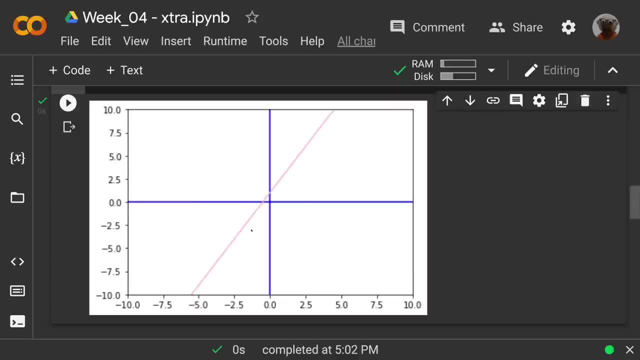 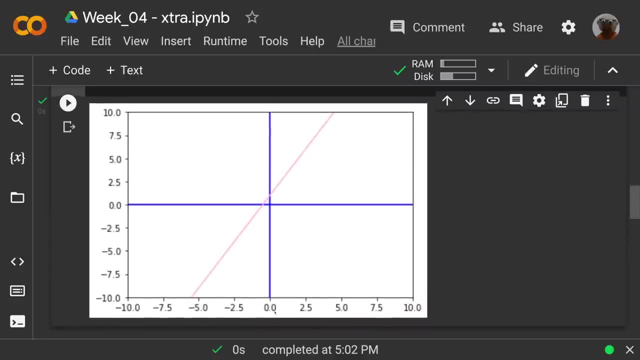 We'll see that in a second here. So there we go. So we have our axis and our line, But we're, you know, we're not done customizing it. First of all, let's take a look at these tick marks. 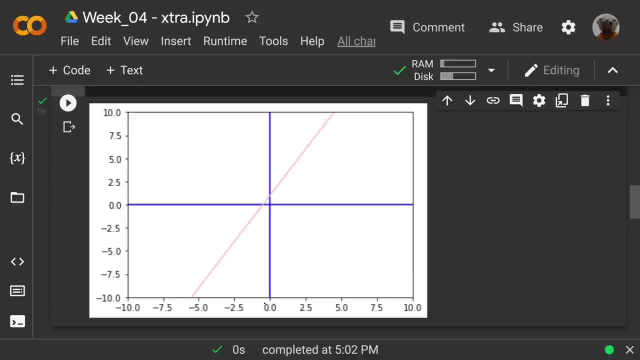 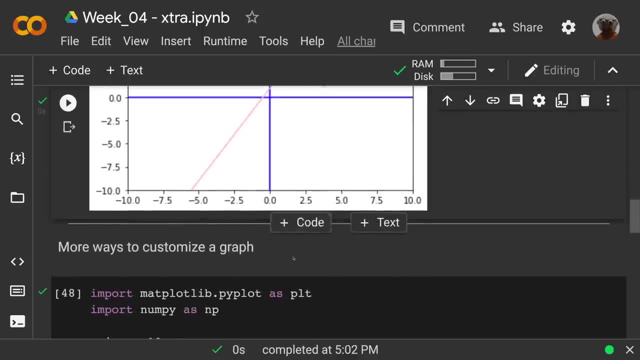 You know, 0, and then every 2.5.. Maybe I don't want it exactly like that. We'll change some of these things and maybe, you know, this seems kind of blank. maybe I want to see the grid lines. 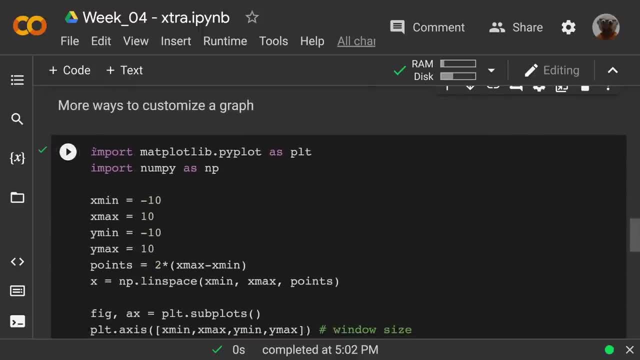 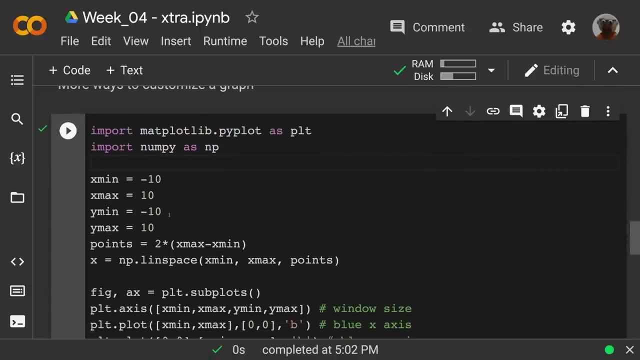 So here's some other things we can do. Alright, I'm still going to import, certainly, matplotlib, but I'm also doing numpy because we use that for some of the things for graphing, And same thing. I'll define you. 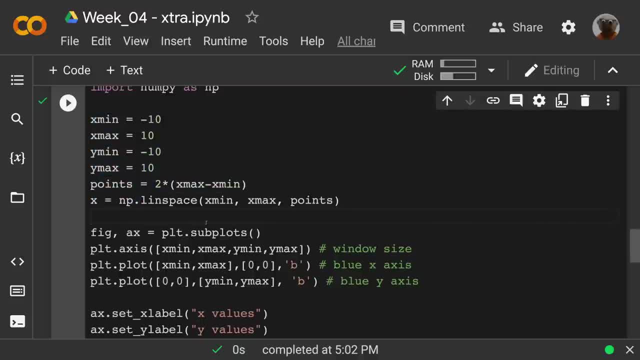 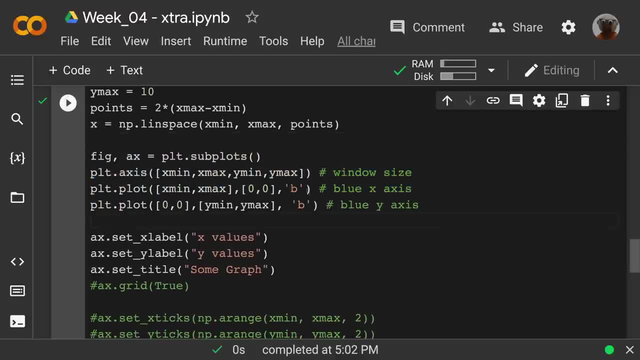 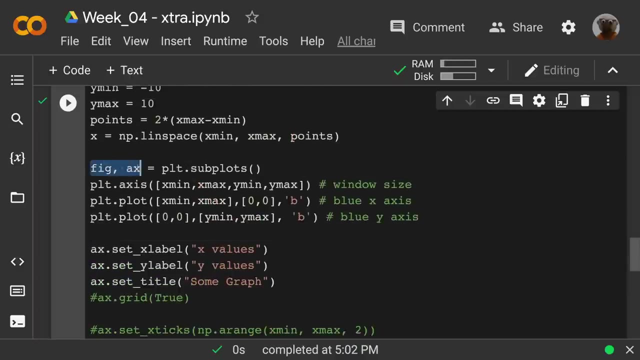 know the window up here and the x values based on that window, So for now I'll keep this. you know the same axis, I just like blue, so we'll keep that. Now notice when we do up here figure and. 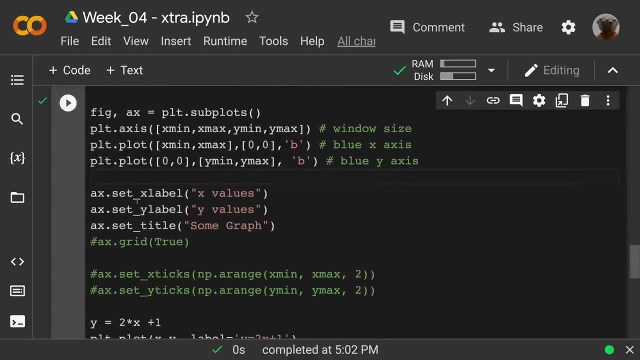 axis, so the labels would be in the axe variable. So axe dot set x label. axe dot set y label, axe dot set title. There we go: x values, y values and some graph, And I didn't mean that. 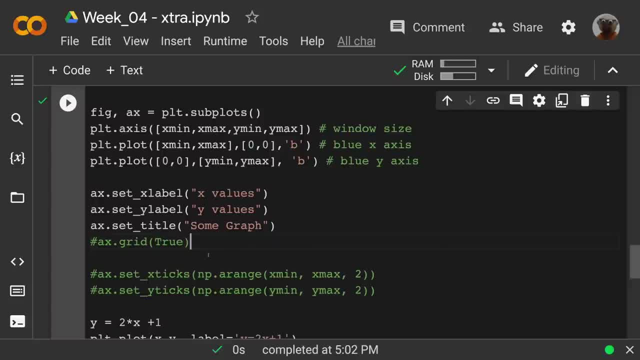 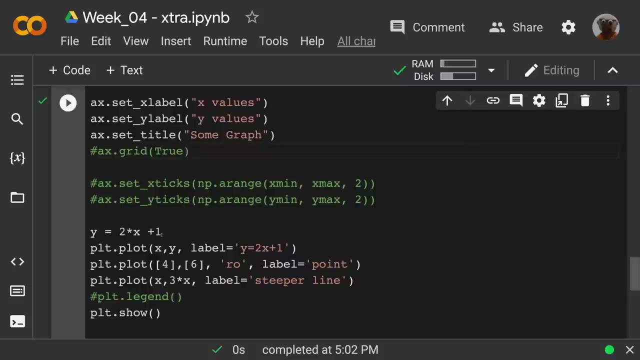 some graph, like whatever. I meant more like you know, like from Charlotte's Web, some graph, So anyway, so we have these and I commented these out. we'll get to these later- and I have a few other things here. 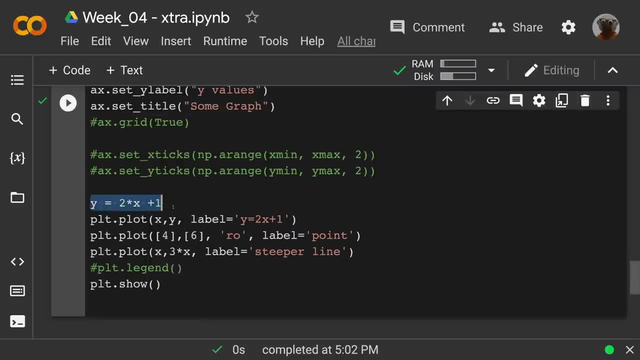 So I still have one y value, and then I'm going to plot that. Now, notice this, I'm going to define this as a label. You know, it can have a label rather than a color, but notice no color. I can also do a color. 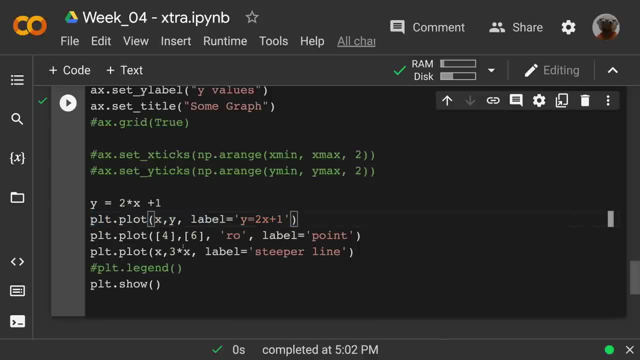 but since I don't have one, we'll see what color Python assigns to us. And then I decide to plot a point, and in this case it's red, and see zero red, or that's actually o the lowercase o so 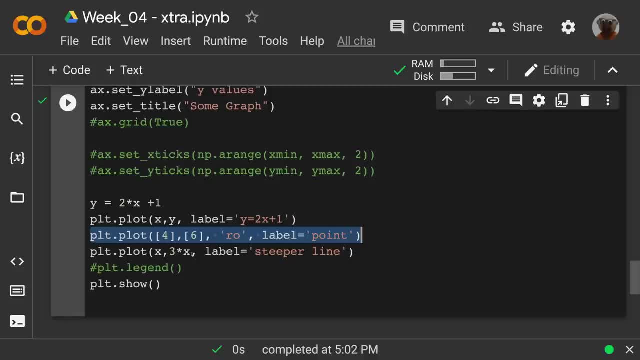 it's going to be a circular point, and then this one's going to have a label too, And I'm going to plot something else- here's same x values- and then notice I can define the y value up here and then say y, right there. 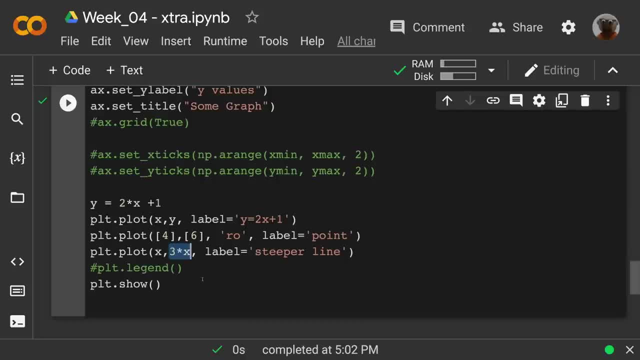 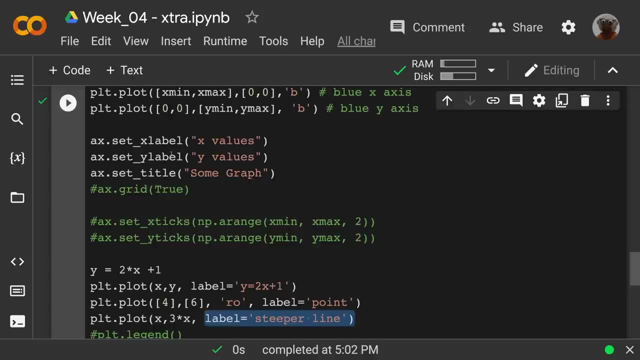 or I could put the y value in here directly. Either way, whichever you feel like doing, I wanted to show you the different options here And again, we have this label also, So let's just take a look at the x label. 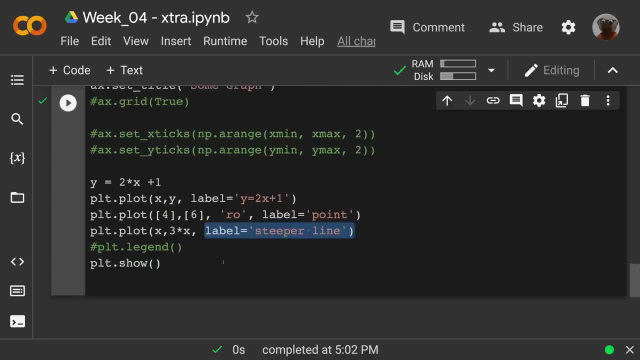 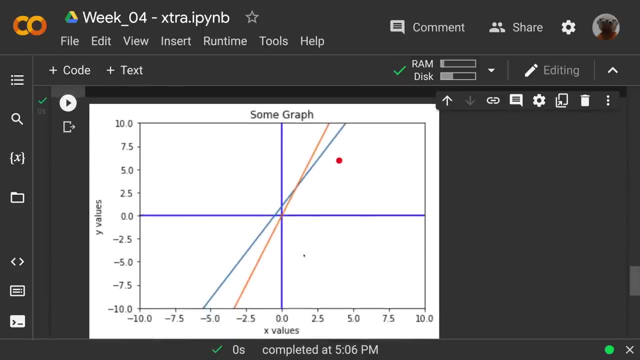 the set, x label, y label and the title, and then we'll see these different, these different lines. So there we go and you know, we get nice orange, a different shade of blue, and I define that as a red dot. 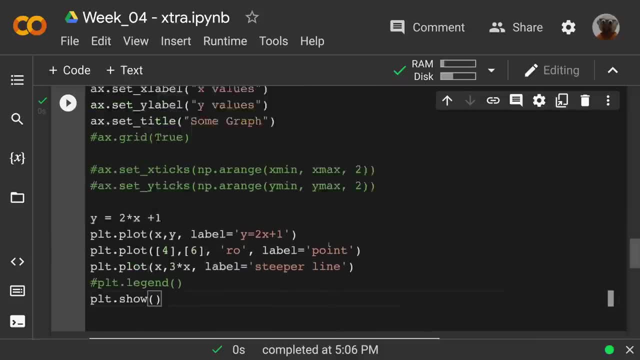 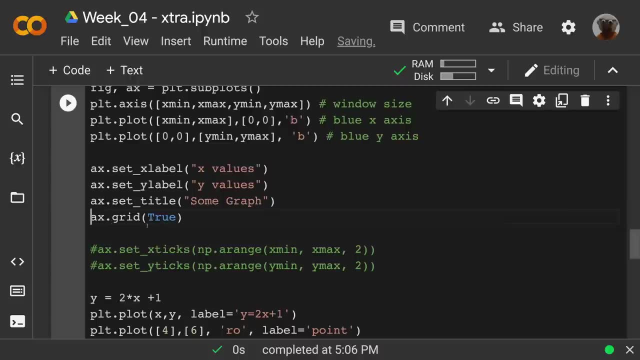 So there we go. But what if? alright, so let's see. What if I want the axis to show the grid? It looks kind of plain. What if I want to see the grid? So when I comment that out and this: 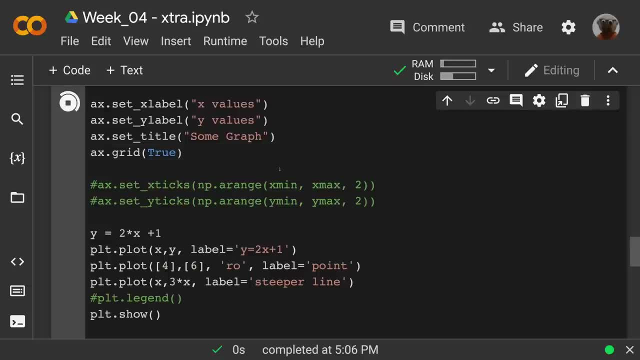 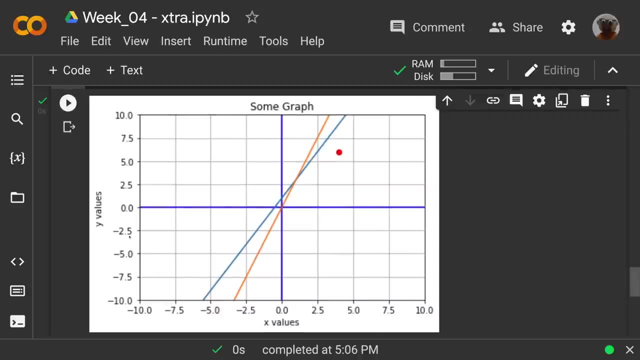 one notice true is a capital T. It will actually show the grid lines and, you see, it does line up to the tick marks that are already there Every 2.5.. But there we go. So if we want to see, 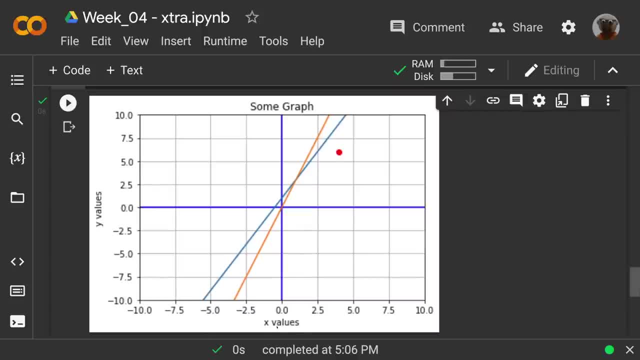 the grid lines and we have this. and now we have our x, you know, our labels- x values, y values, some graph You could actually put the graph and in one of the later units we'll look at some details about how to. 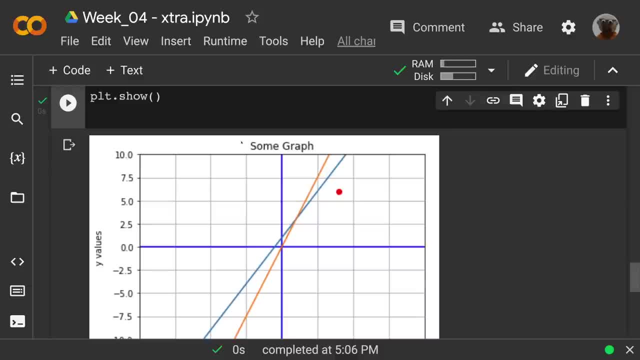 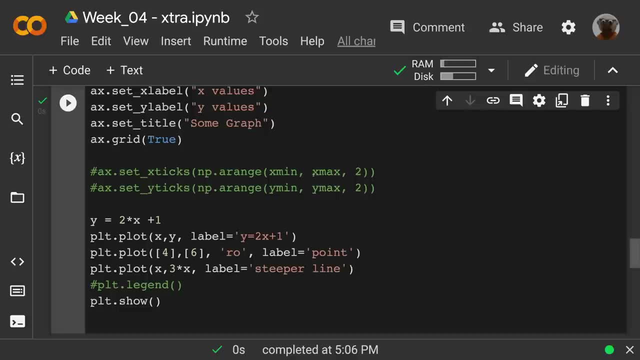 even automatically, if I wanted to graph one line and have the title of the graph be that line. But you know, you could always just type that in. You know, instead of some graph, you could actually just type that in as a string. you know the equation. 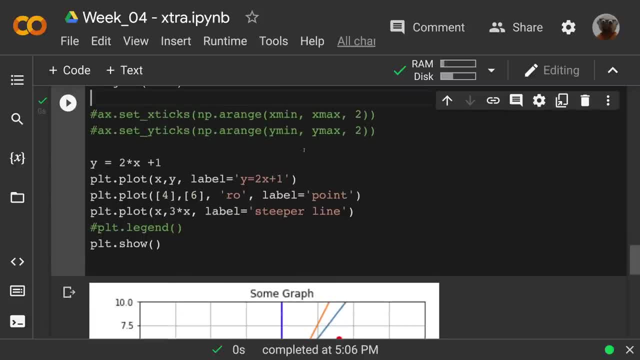 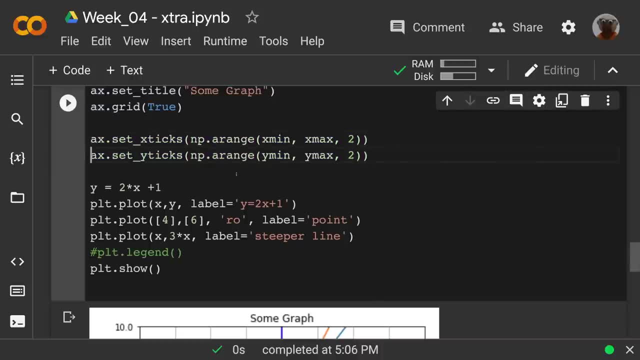 of the line Okay. so let's take a look at NumPy again And in this case let's say, the 2.5 in each direction is not really what I want. So again, we have x dot and we're going to set x ticks. 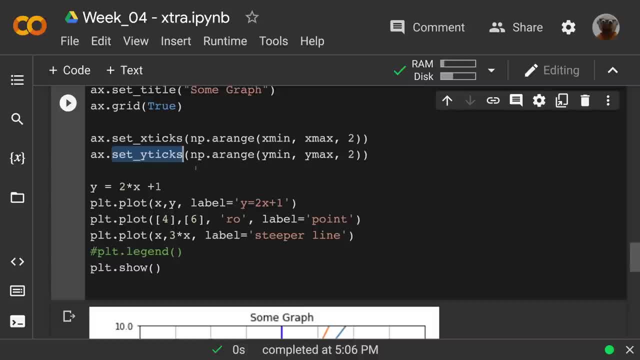 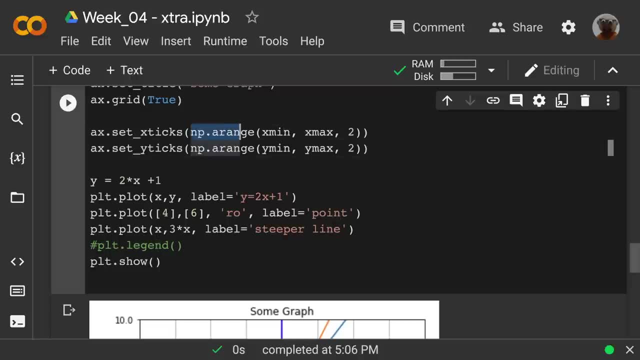 and set y ticks. So we're setting these tick marks on each axis. So it's a different sort of array. I'm going to do nummparrange And what do I want to arrange? Very similar to the way we did. 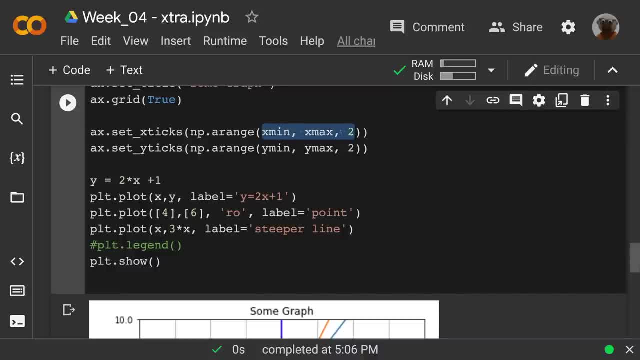 x values, I get my minimum, my maximum, and then this is: how often do I want to tick mark every two numbers? So that's what we're going to do, from ymin to ymax And you see, again basing it off of those original variables. 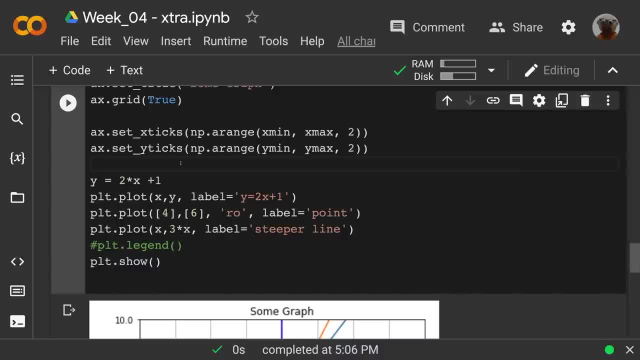 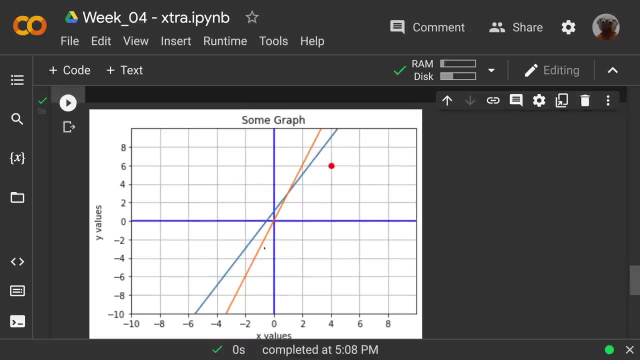 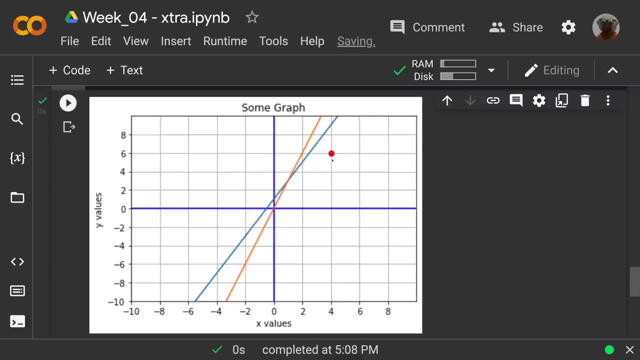 if the window changes, then all this will update automatically. So there we go. So let's just take a look at that. Supposing I change the tick marks And we see then now every two- And maybe that's a little bit better- instead of 2.5. 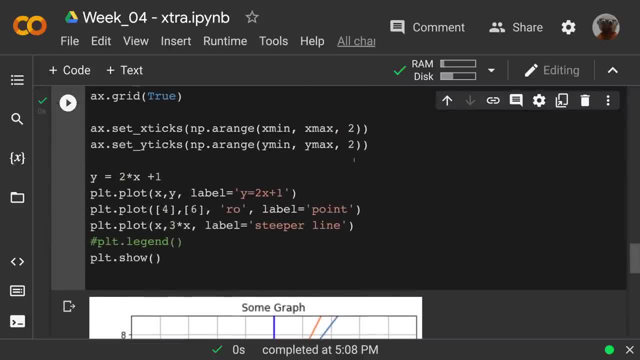 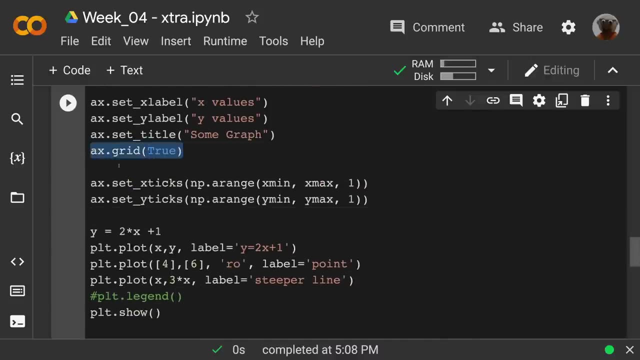 And we see these Now. if I wanted it every one, then I'm going to change that just to one. And notice, this is just for the tick marks along the side, But up here, when we do xgrid, true, that's going to just follow whatever tick marks we've assigned. 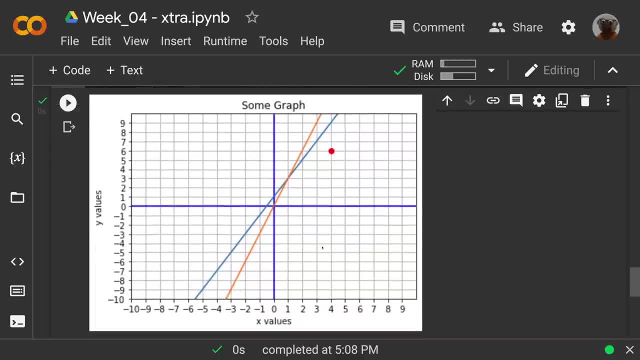 So now we just change this every one, And now we get this sort of graph where I definitely can count the boxes and see. You know, let's take a look at the slope of each line, Let's see these, And Python still does it around the edge. 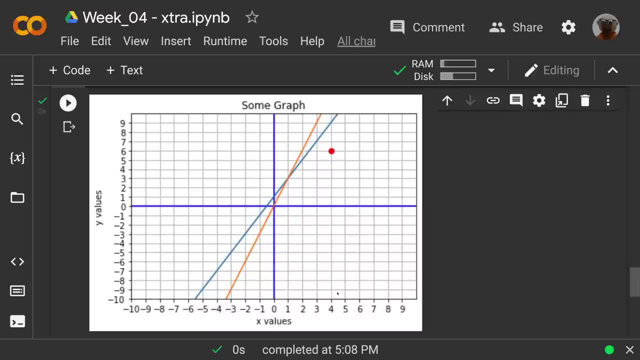 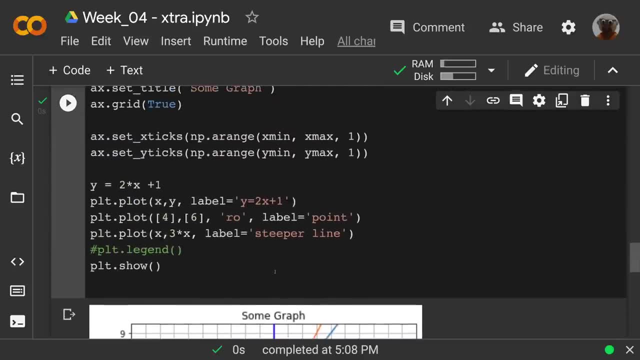 So that way it doesn't get in the way of anything that's in the middle of the graph. Alright, there we go, So we can keep this. That's pretty nice, Okay, so what's one of the other things? 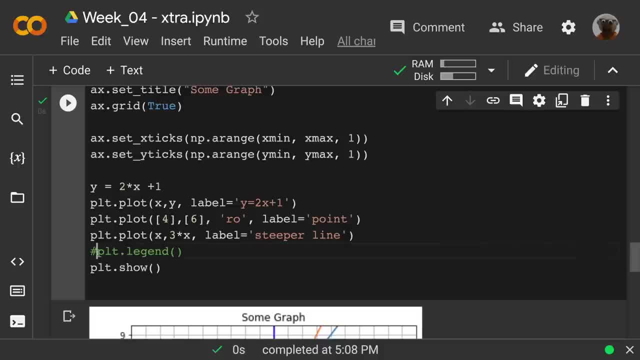 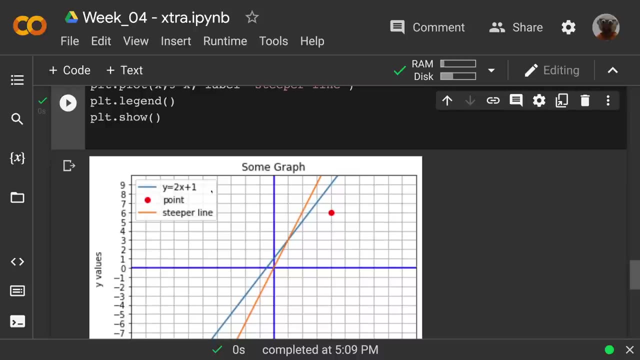 We have all these labels but we didn't see them anywhere. So if you have all these labels, then we add this other PLT dot legend. There we go And we can see these labels. So I wanted to show. 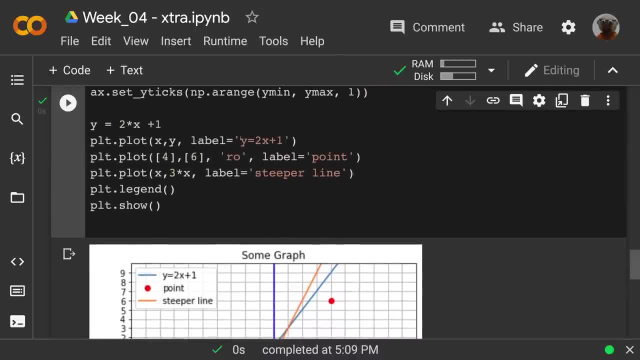 you that each of these labels we can have. you know, this line we labeled with the equation, The point. I just wrote, the word point, but you could put anything. And the other one labeled with just some words, steeper line. 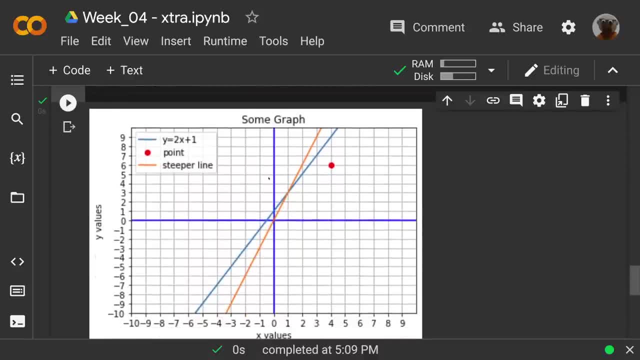 So we could always do this and in the same way, you know, even if Python assigns it, you'll see the matching. you know which line are we referencing, which point are we referencing. So some good things that we can do with these. We can. 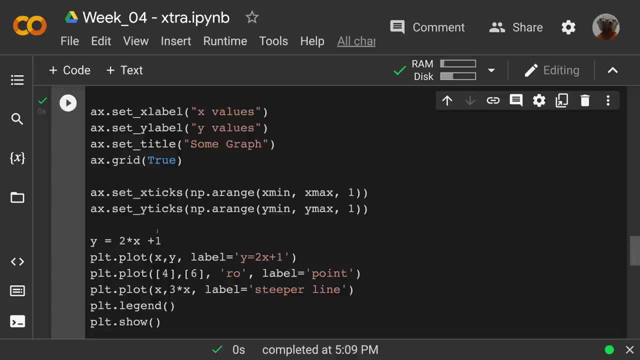 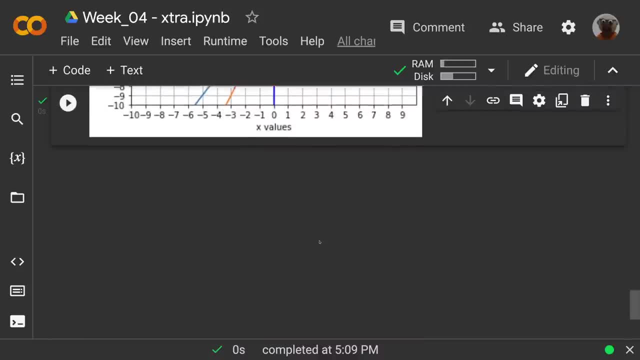 have the tick marks or not. We can change how often they come up. We can have the grid or not. We can change these labels Alright, And I encourage you just to get in and you know, tinker with this. 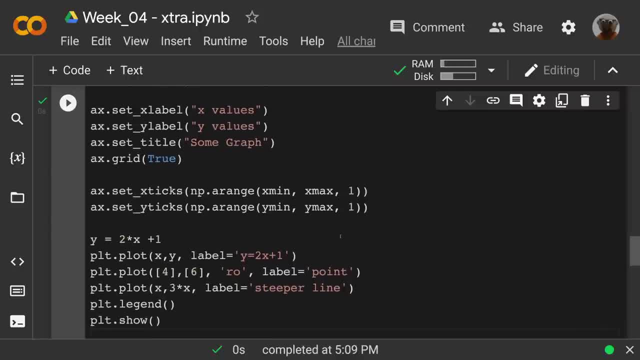 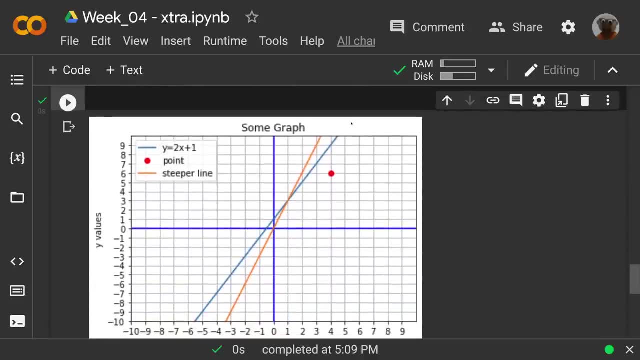 You know, take a look at some of the different ways that you can, you know, match up different graphs. You can, you know, set different things, And we will get into even more graphing, but that's going to be when we get to. 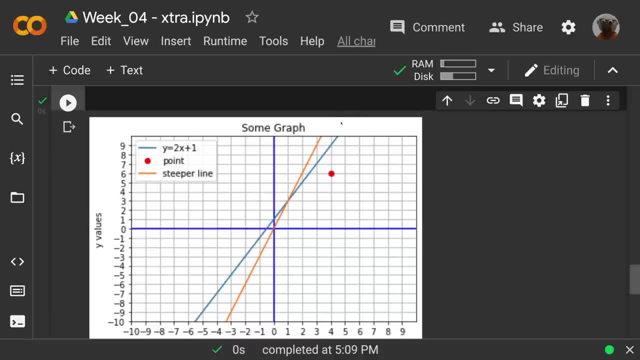 you know systems of equations and some other more complex graphs. So then we'll revisit this and then we'll, you know, go a little bit deeper, Try a few more things with the graph, But I think this will get you to be able. 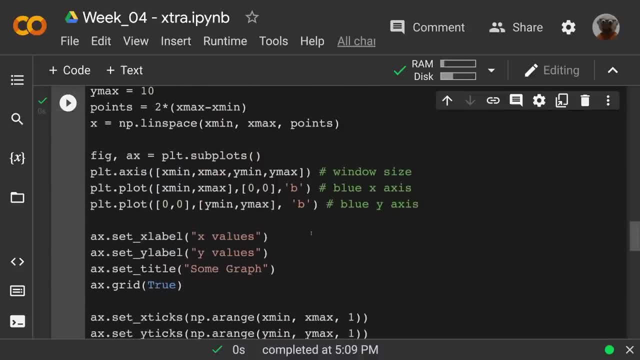 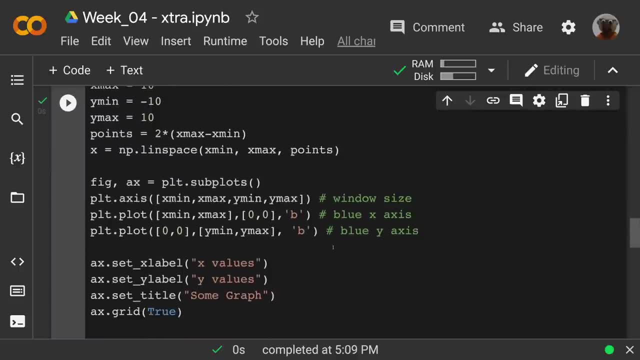 to display any function you have and, you know, hopefully display it in a way that you say, yeah, this is exactly how I wanted it to look. There you go Customizing your graph, Alright. So, yeah, get in there and tinker with. 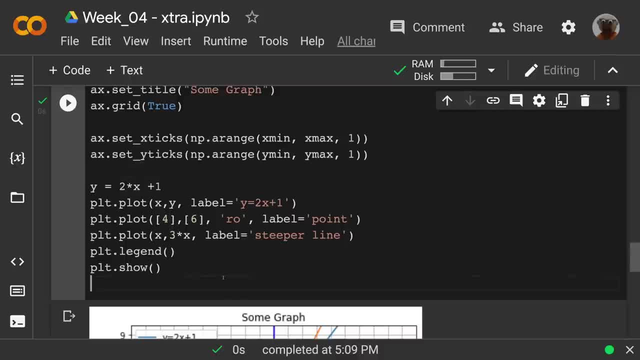 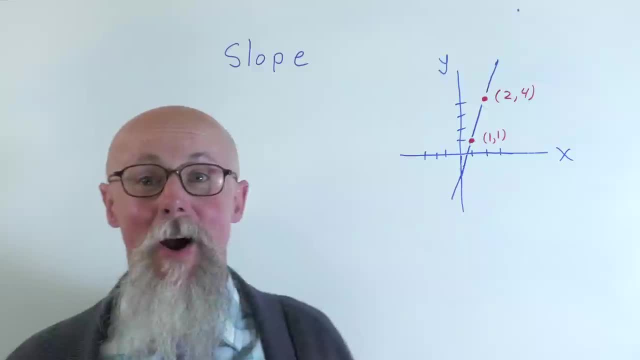 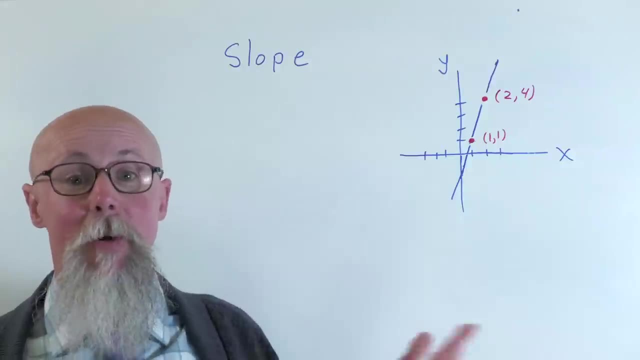 this and see different ways that you can change the graph. So let's talk about slope. How can I describe this line that's on an angle, using, you know, describing how it goes up and over. So that's what slope is: Picturing these lines. 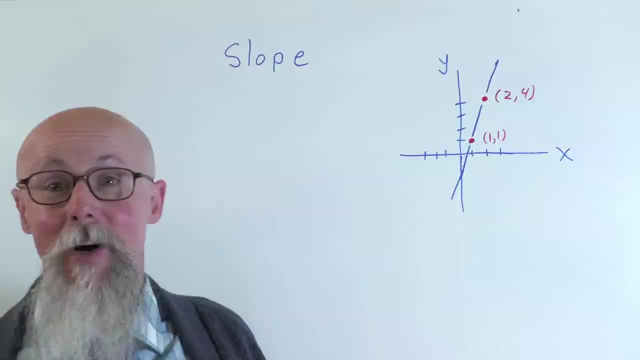 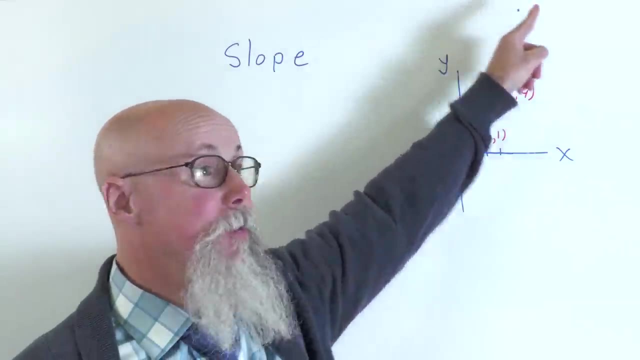 that have a slope to them, that they go on some sort of angle, but we're going to describe them going up and over like steps. How much am I going up and how much am I going over? Up then over, up then over, like steps? 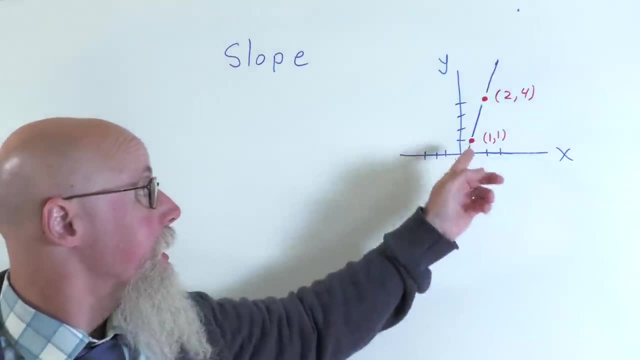 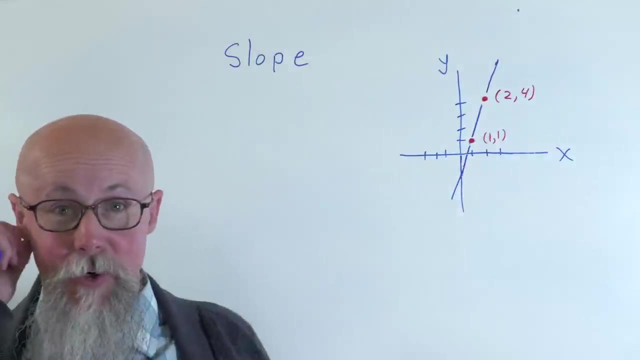 So if I have two points and if I have the graph that I'm looking at, that's great. I can just count. You know, looking at two nice points that work out as integers, that makes it easier to count, So I can say: 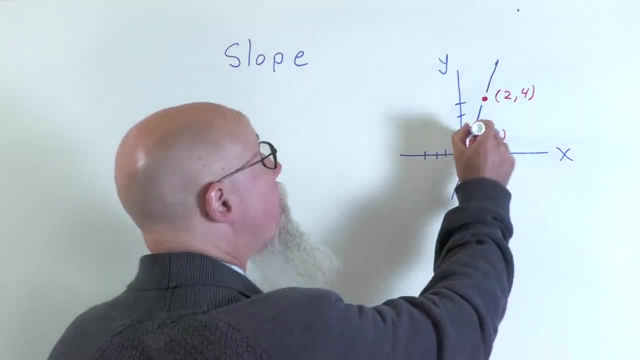 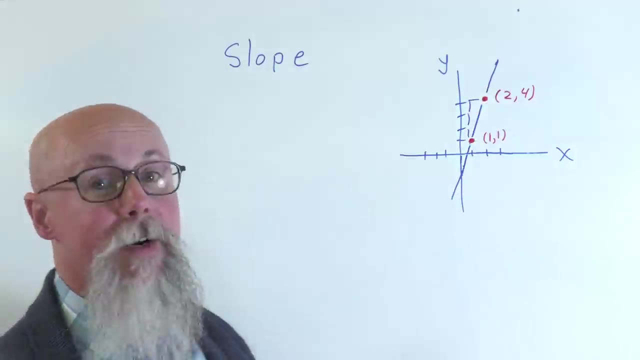 from this point to this point. I'm going up three, one, two, three and then over one. So up three over one. well then, my slope is three And I can do the same thing, you know, from that to the. 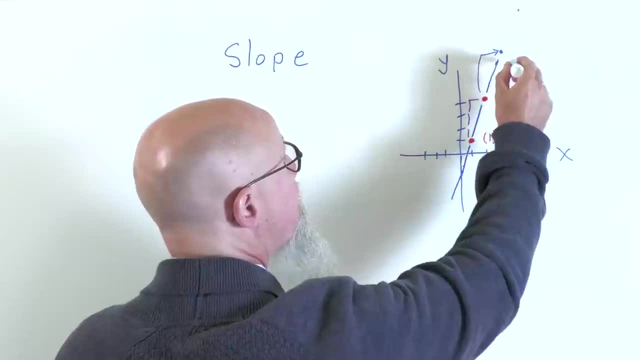 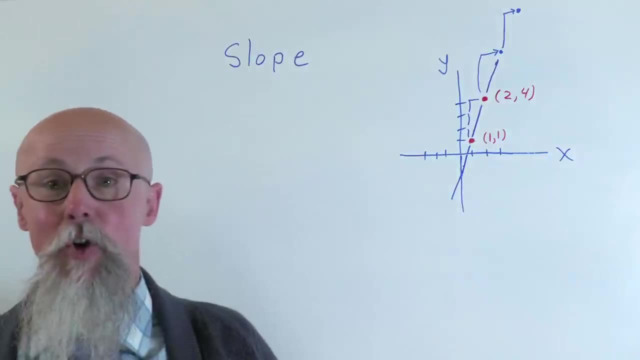 next point. I can go up three over one plot a point, up three over one plot a point, etc. And it would be the same slope anywhere on the line, because it's a linear equation, It's a perfectly straight line. 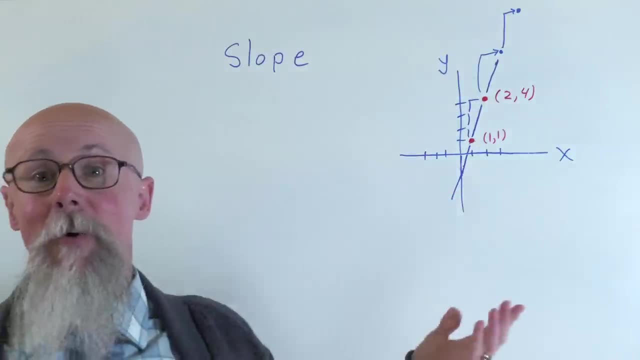 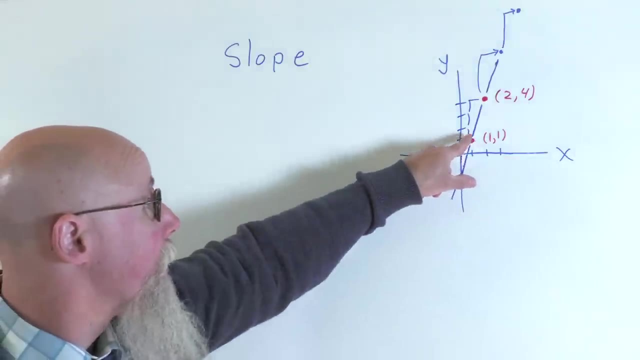 So that's great, I can count If I don't have the boxes or you know, just have things like this. but if I have the points, that counting that, how much am I going up? that's the change in y, because y tells me if I'm going up. 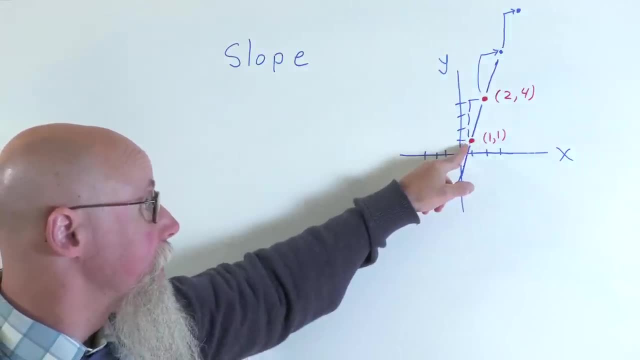 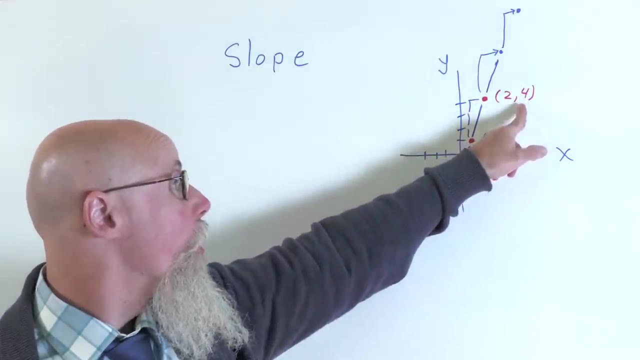 or down. So if I look at this, I'm going up. I just counted three, but I could also subtract, taking a look at the y values, Four minus one, or then how much am I going over? and it's always over. 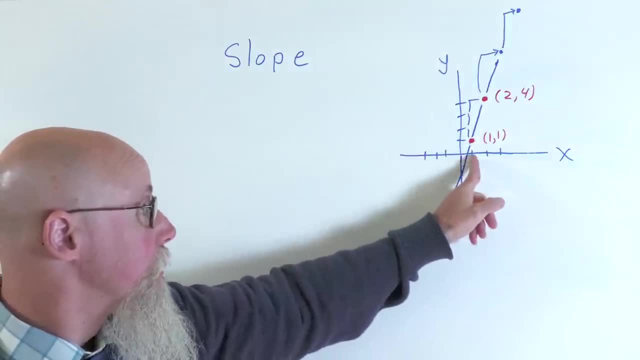 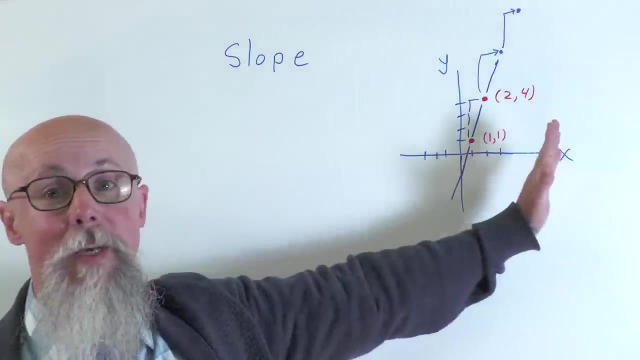 to the right, So I can look at the x values. So from one then to two, two minus one, how much am I going over? So it's always over to the right. In this case it's positive because left to right it's going. 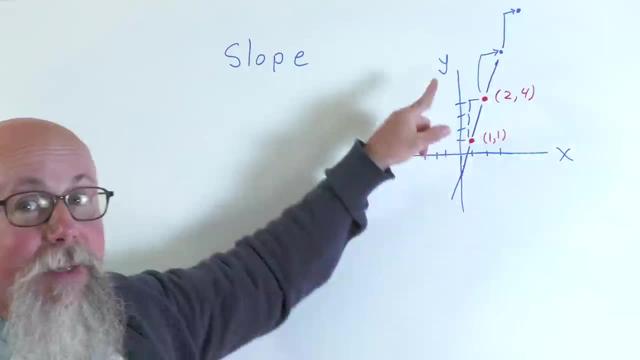 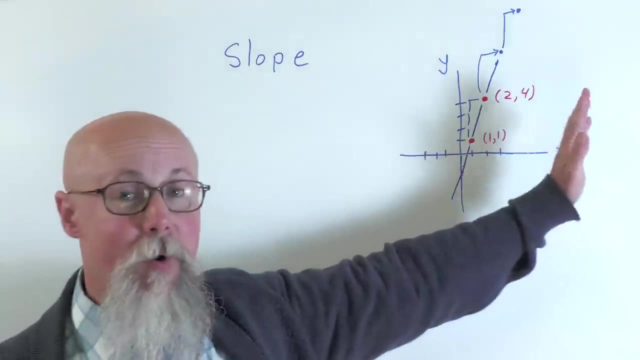 up. If it was left to right going down, then my second y value would be less and when I subtract then it'd be a negative number. So it's always going to the right. but y would be positive if it's going up or negative if it's going. 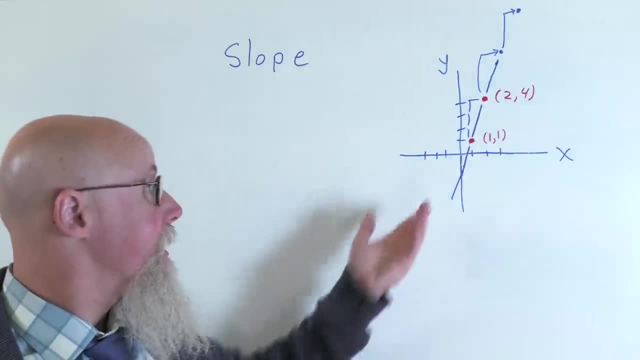 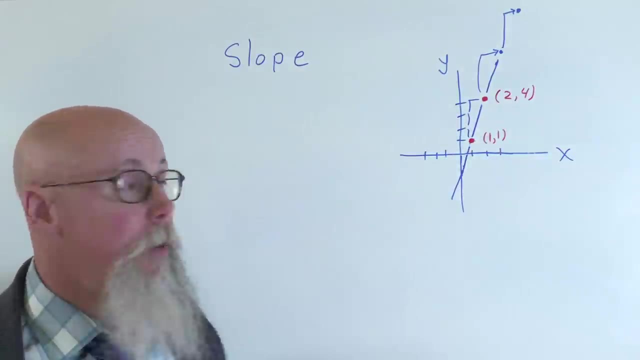 down And so if I had these and I can count, but looking at this I know I can subtract. So what's that formula look like? Well, I can write out the formula here: slope m equals and that's right. 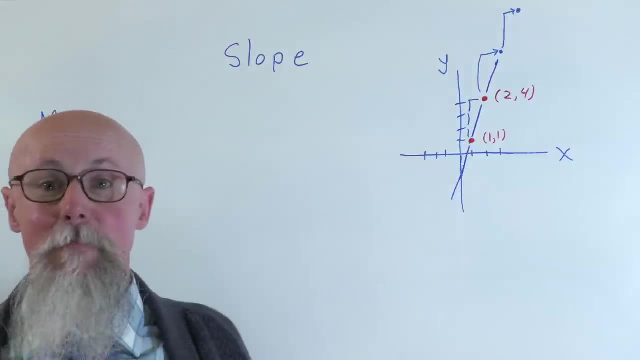 m for slope because it's how much we move on the graph. So somebody started using m and it caught on. so we're going to use m for slope. it's how much we move on the graph. And remember I said it's. 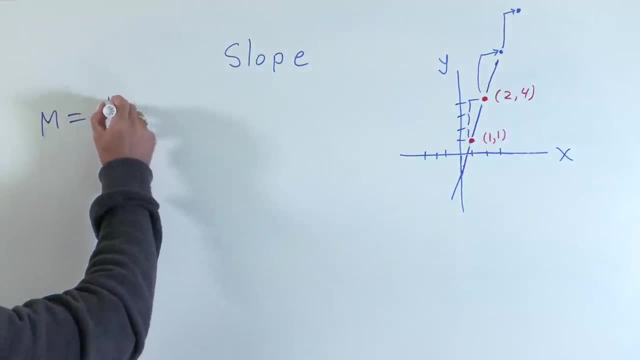 how much am I going up? so that's the change in y, and I can subtract that y2 minus y1.. And so I would use a little subscript. you know y2, y1, and that indicates my second y value minus the first one. 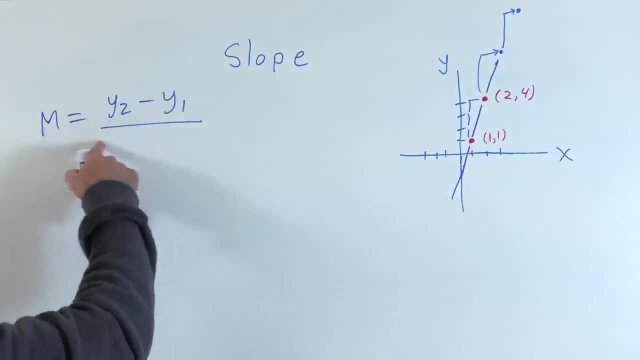 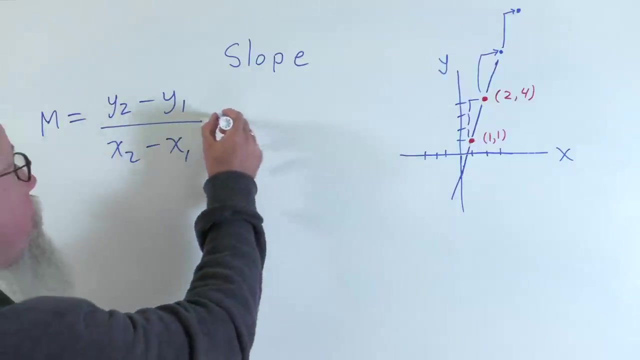 Then the change in x would be very similar: x2 minus x1, and again the subscript for the second x value minus the first one. Okay, so now that I have this formula, let's plug in these numbers and see. So we'd have 4 minus. 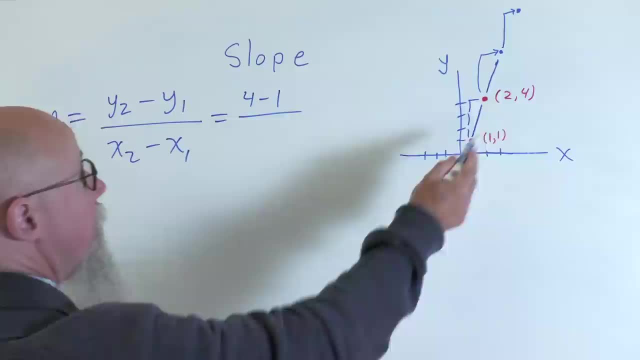 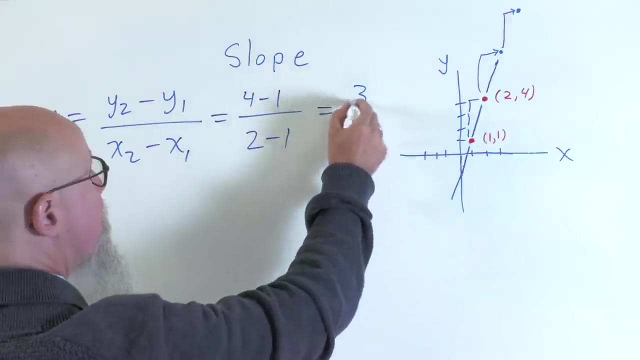 1, 4 minus 1, I'm subtracting my y values- and then 2 minus 1, subtracting the x values, And what do I get? 4 minus 1 is 3, 2 minus 1. 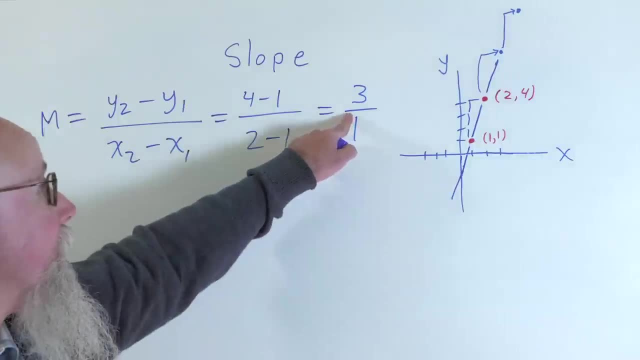 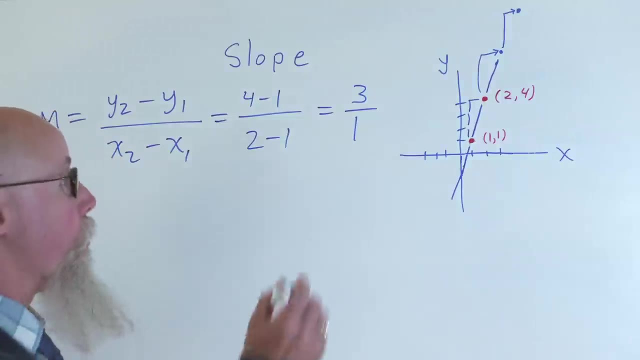 is 1, and 3 over 1,, any whole number over 1,. you know, divided by 1, it's a whole number. I don't have to write over 1, so I can just write 3.. So that's. 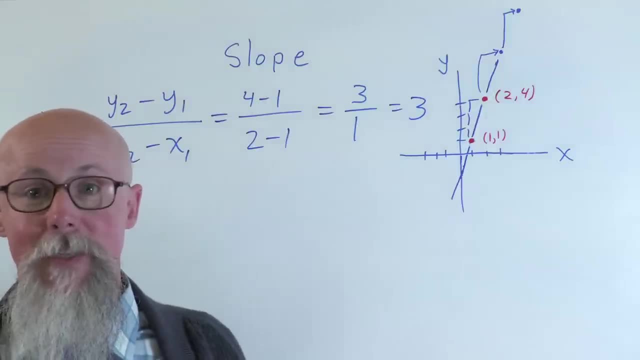 where anytime we see a slope, that just is a whole number, it's that number over 1.. And there we go. So we have counting, if I have the graph subtracting, if I just have these two points- and you know I'm using that- 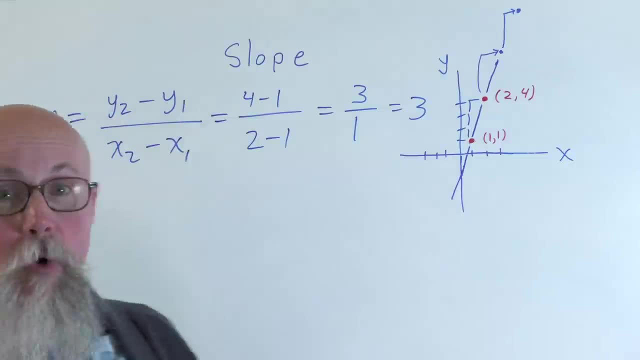 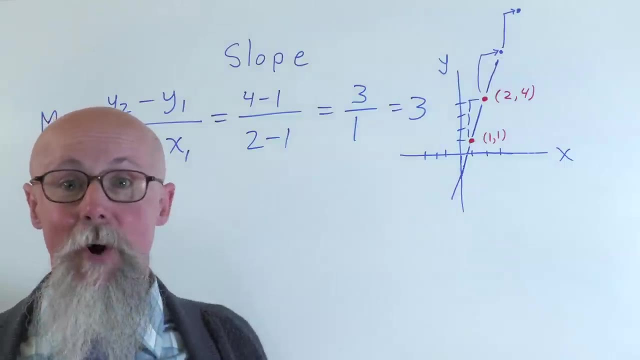 formula. So this is great. It's the same formula you know, anytime we have slope for a linear equation. So let's take a look at how we can turn this into code, because I want you to get into this mindset that anytime we have a formula you can. 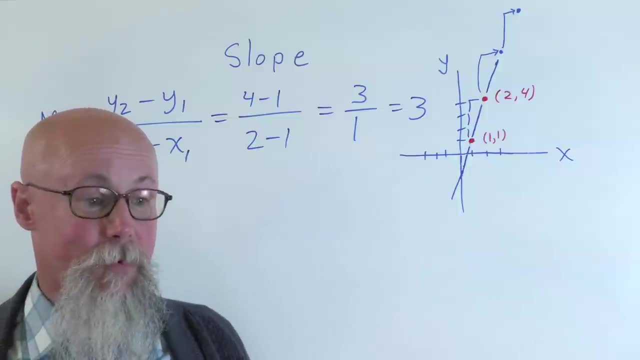 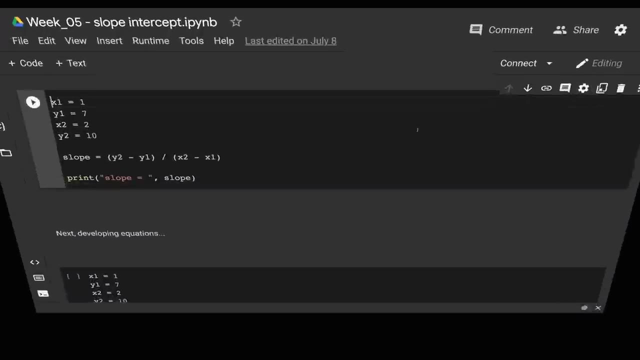 write a program for this. and you know, there we go: Input the numbers and output, in this case, the slope. So let's take a look at the code and we'll see how we can do this. Now this part. 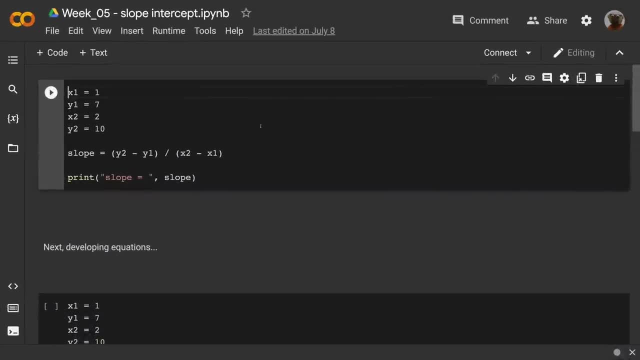 is going to be brief because I just want to show you that you can connect any formula you know. here we're going to define our x1, y1, x2, y2, and put that into the slope formula. Slope equals y2. 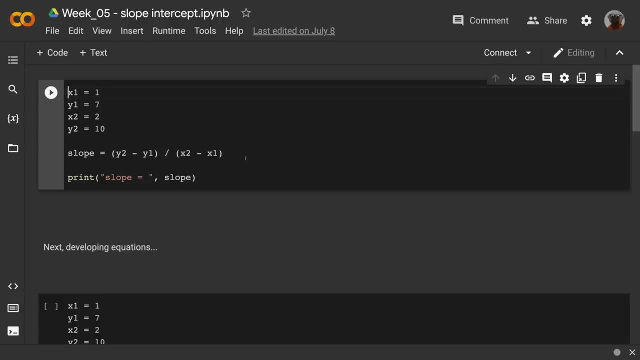 minus y1, divided by x2 minus x1.. And really, then this is a useful formula, and others you can just define your variables and run it through the formula. Here we're just going to output the slope. 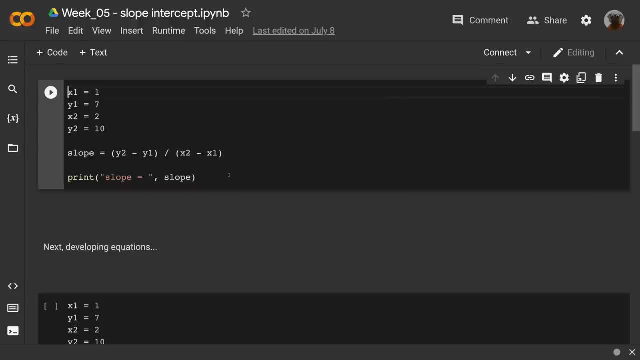 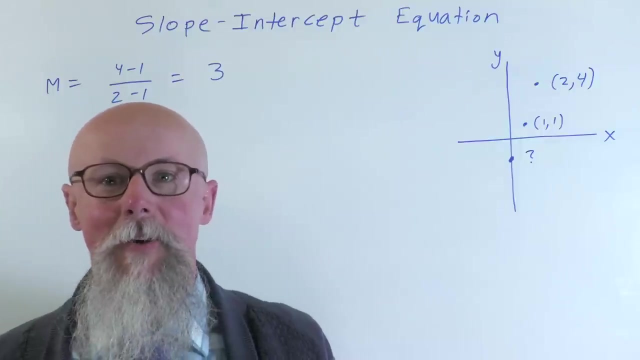 There we go. All you need is the two points. Next we're going to work on developing the full equation, but then let's take a look at how that comes together on the graph first. Alright, so we've already figured out that the 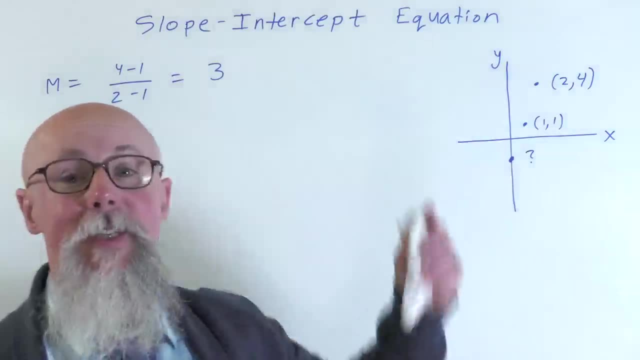 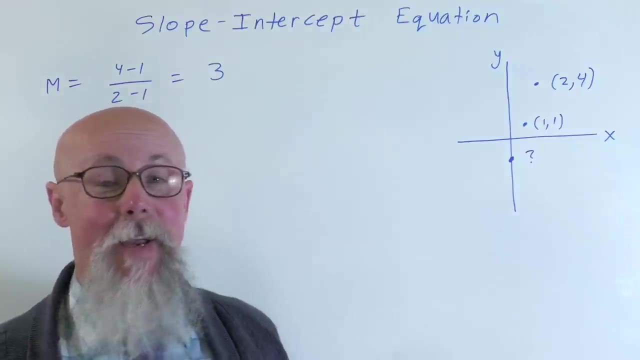 slope is 3, in our two points. but let's say we have these two points and we want to figure out the equation of this line. We know that this is linear and I have these two points that we've figured out, that the slope 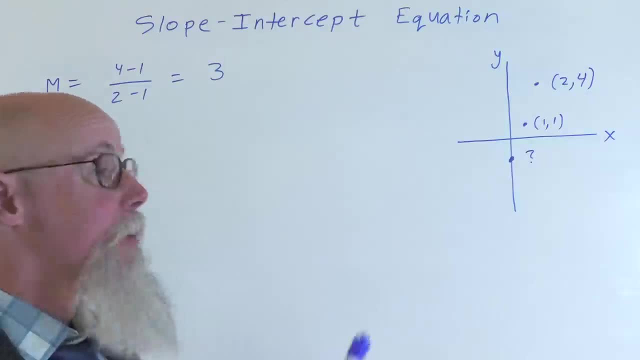 m because moving it from one point to the next, we went up 3 and over 1, or I just subtract 4 minus 1 over 2 minus 1, and then 4 minus 1 is 3, 2 minus. 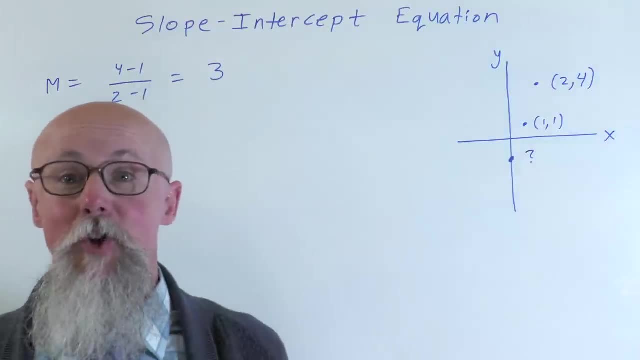 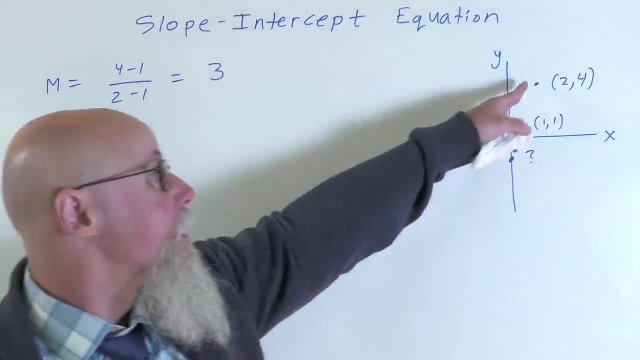 1 is 1, so 3 over 1.. We figured out that the slope is 3, and we want the full equation of this line. Now, knowing that it's linear, we can imagine here that it would cross the y-axis somewhere. 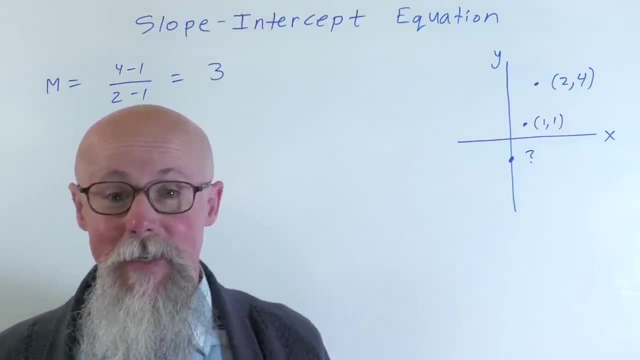 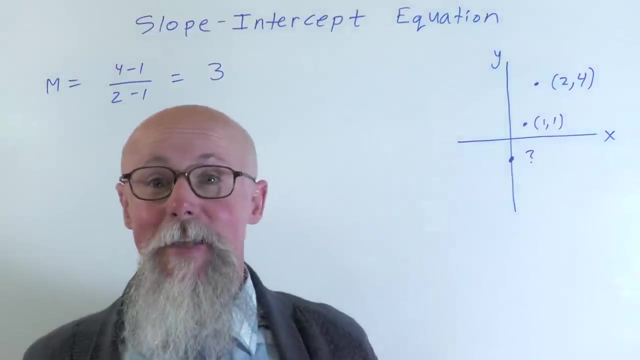 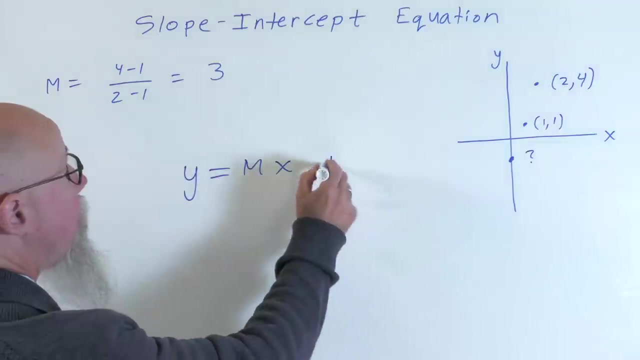 and that's what the y-intercept is. The intercept is: where does it cross? So we have a nice formula, slope-intercept form, and that slope-intercept form is y-intercept. y equals mx plus b. Now we called the slope m because 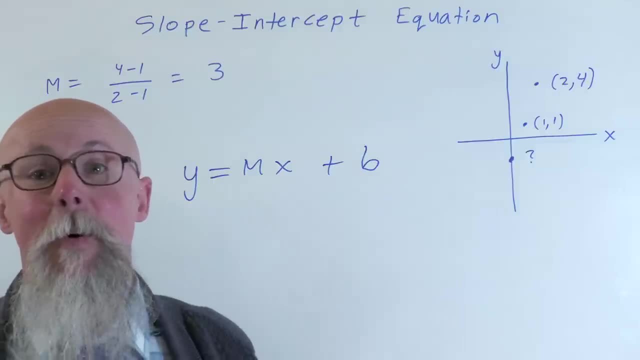 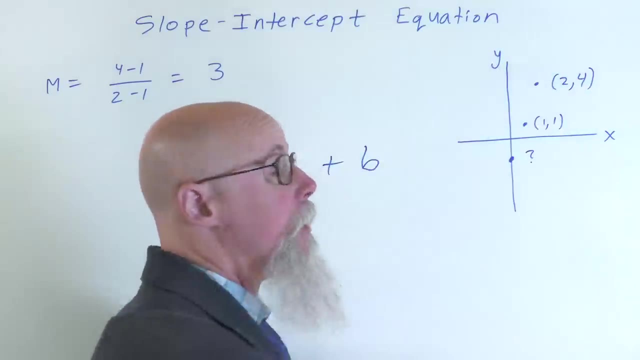 that's how much we move from one point to the next, and we'll call the other one b, because that's where we begin on the y-axis. So many things happen in this first quadrant, where everything's positive, so we picture that we begin on the. 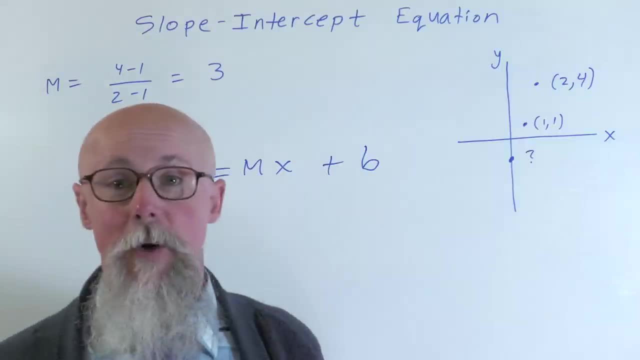 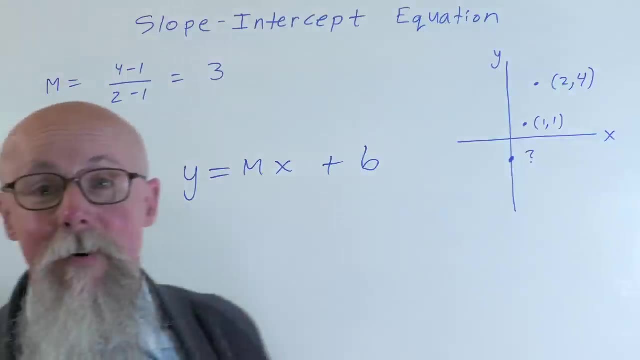 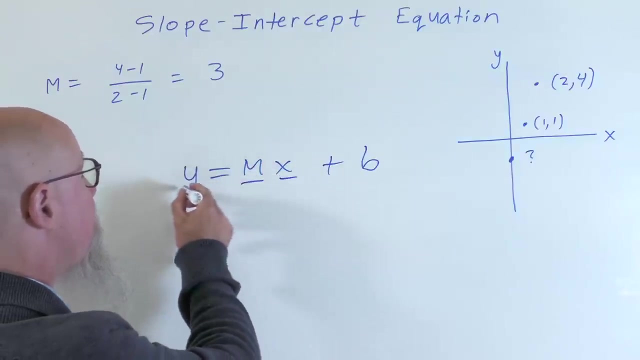 y-axis and then move in that direction. Of course, you know we can go in different directions, but so I have this: y equals b, equals mx plus b. Now what we have is our slope is m, The xy comes from. 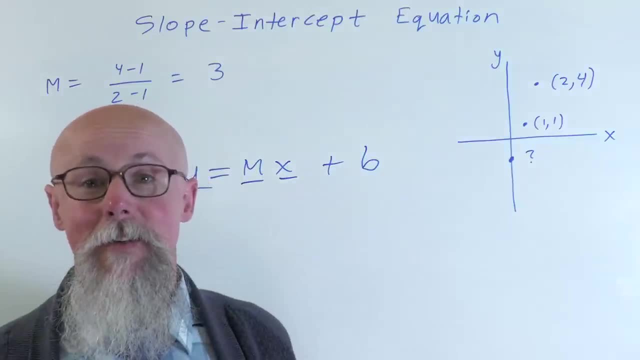 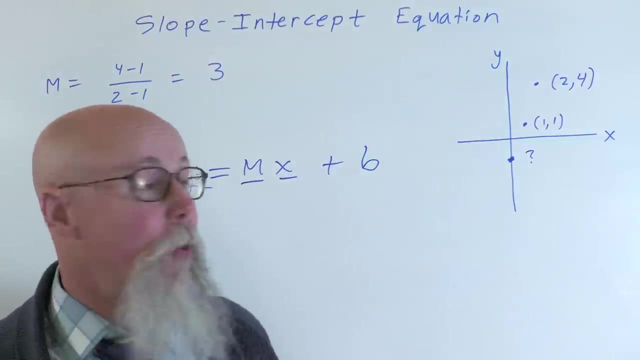 any of these xy points. So I'll pick one of these points and then b would be the y-intercept. It works out that way. So if we take a look at this, I'm going to take one of the xy points. 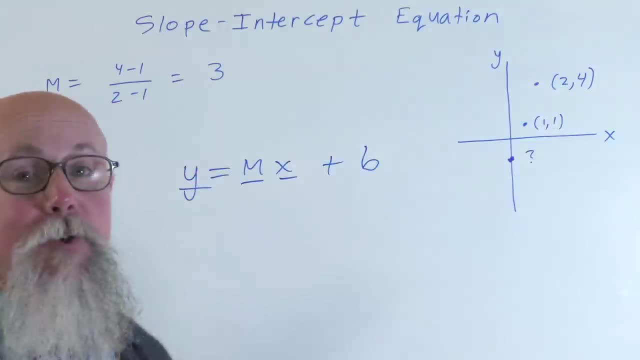 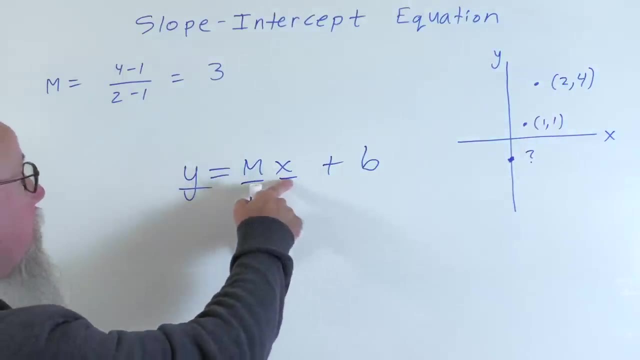 How about I take this first one here, because it's one that'll be nice and easy to calculate. It works for either one. So when I plug in this, the y value is one, and then the slope which we just figured out was three. 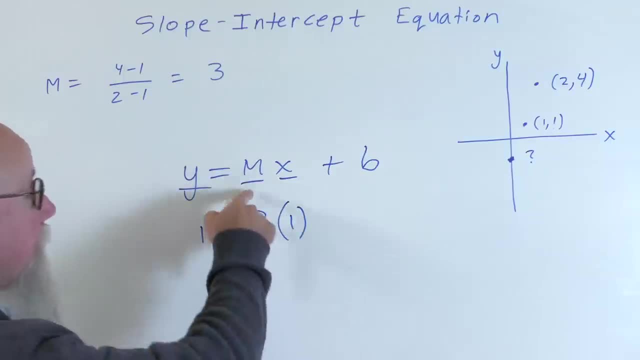 and then the x value is also one. I'll just put that in parentheses. So notice, mx. you know, in my math notation I don't have to write that I'm multiplying just because they're next to each other. So 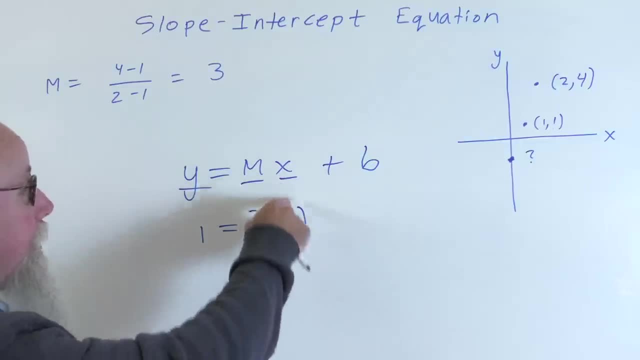 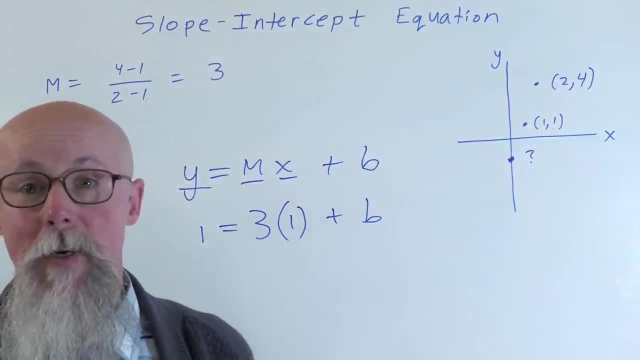 I'll do the same thing when I plug in You know m and then plug in for x and now b, I don't know. So that's where I have. I plug in slope, that I know one point. so that's four things I know. 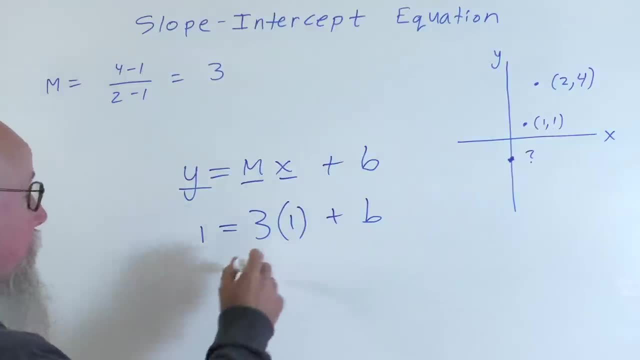 three of them. I can figure out the fourth one, And we'll do this: multiplying one equals three plus b, And remember our one-step equation: subtract three from both sides, so I get negative two equals b. So now that I have this, 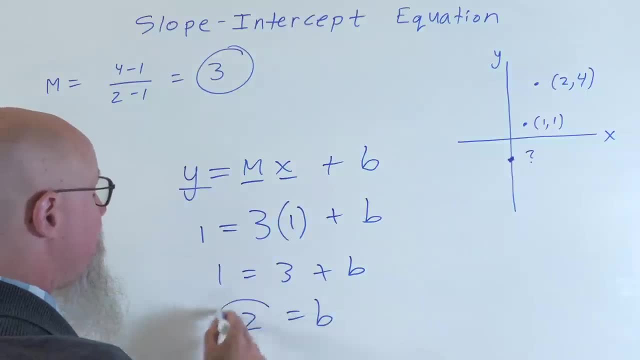 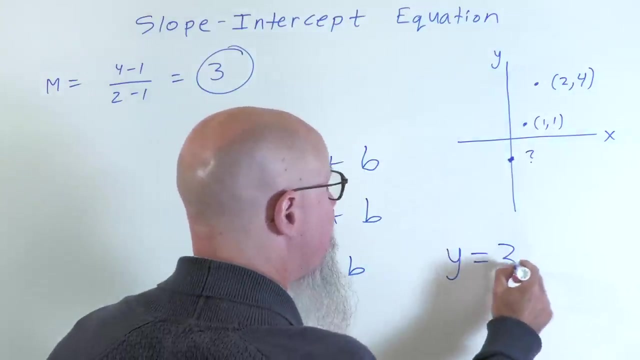 I figured out that the slope is three. I figured out that b is negative two. Then I put it together, leaving xy open, because any xy point on this line will work in this equation. And my final equation is: y equals three x minus two. 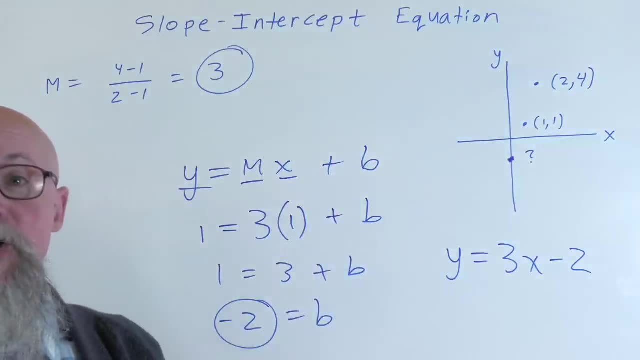 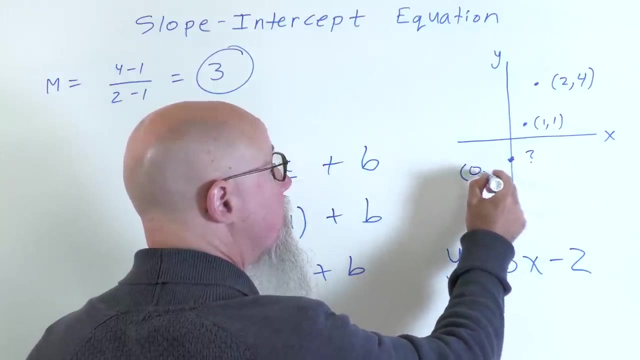 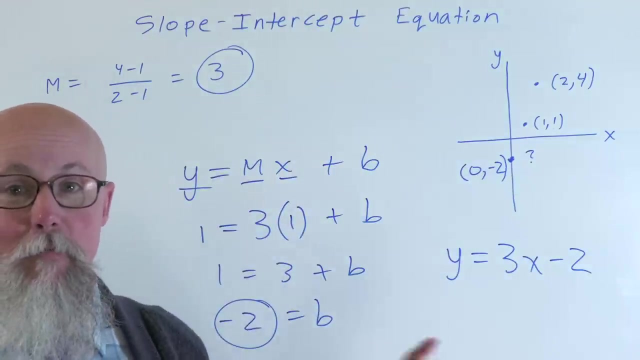 So there we go. We've figured out this slope intercept, and so now I know that minus two it crosses down here, so that coordinate point would be zero negative two, And we can see why. this is why it shows up like this, because 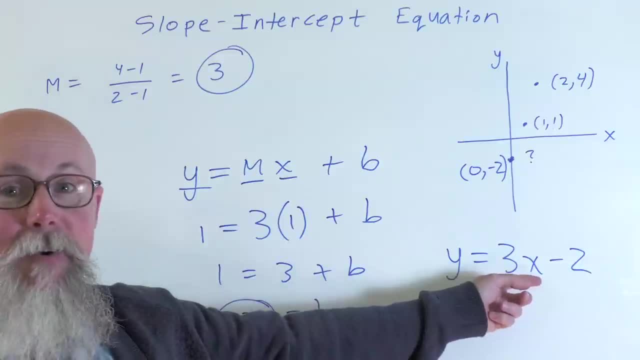 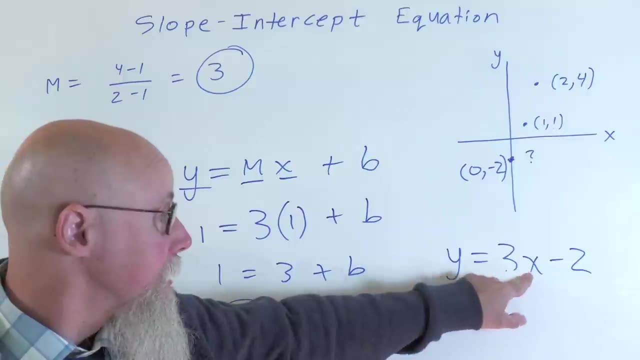 when x is zero, whatever I plug in as an x value, it's going to zero out. So three x, three times zero, it zeroes out. And then when x is zero, that drops out, and then I have minus two. 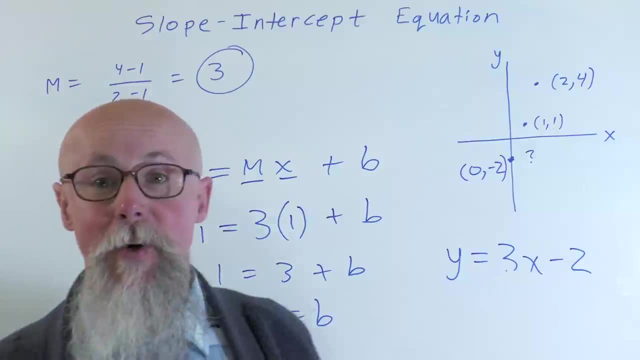 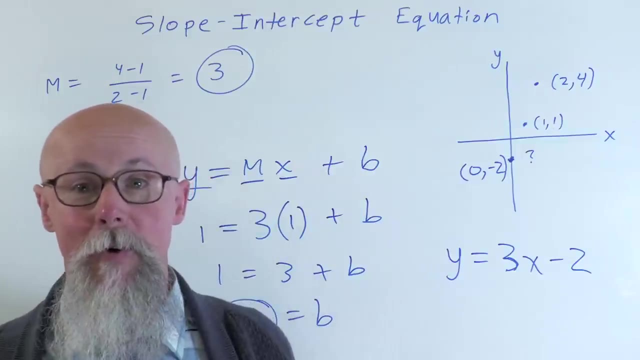 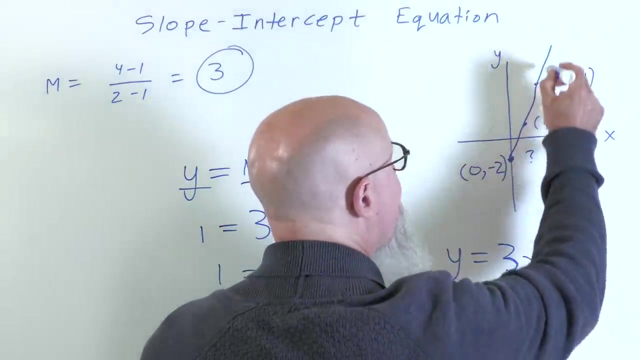 So we see that that works out. So this is our slope intercept equation And we can, when we see this now, if we know the slope, we can generate the slope and the intercept. If I had this line, I could generate that equation. 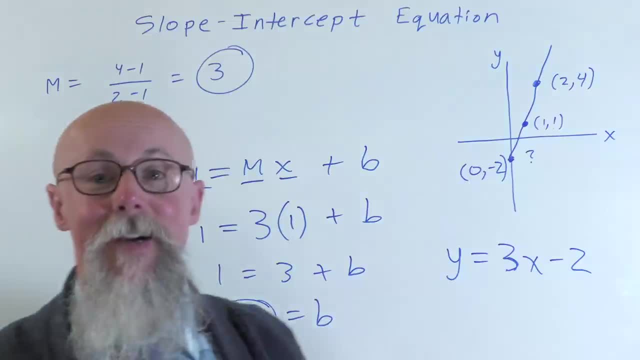 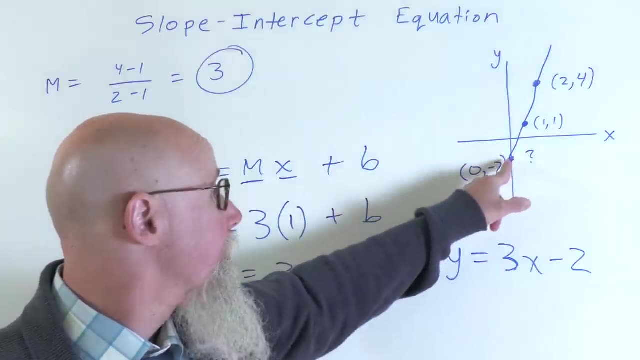 We're going to pretend that that's a straight line, but if I had this line I could generate that equation. Oh, where does it begin? At negative two. Oh, I know that that's b, And then I can count for the slope up three over one. 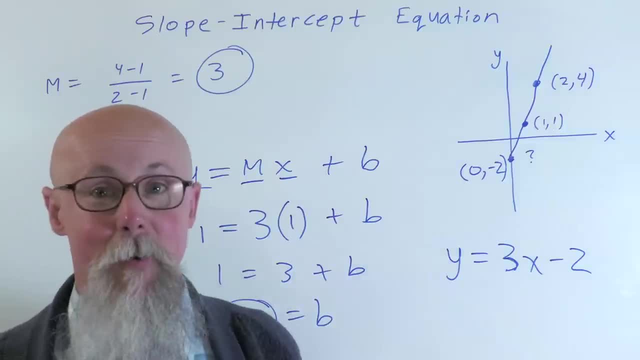 so then I know that the slope is three And I can go the other way. If I had this equation but didn't have the graph, I could say, oh, I'm going to begin at negative two, Zero, negative two. 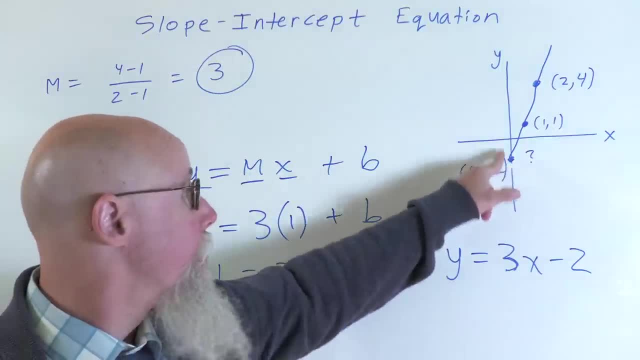 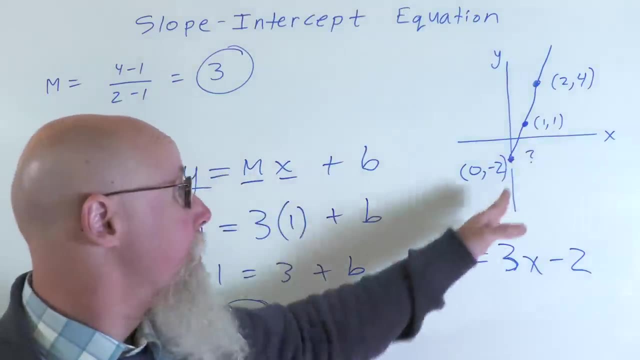 plot that point And then the slope is three. I would go up three over one plot a point, Up three over one plot a point. And if I was doing this by hand- you know paper and pencil- I'd probably plot like three points and get out. 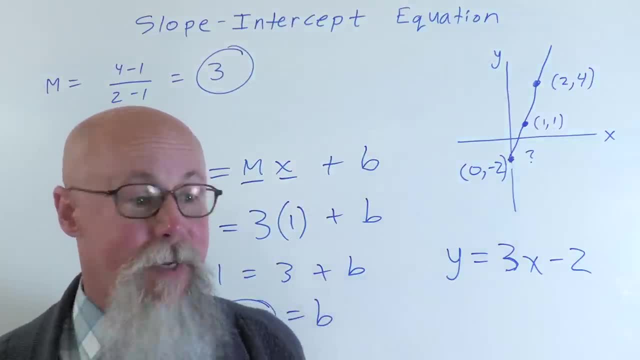 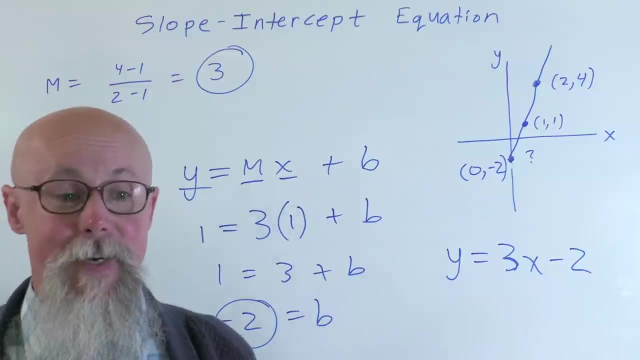 the rule and connect the dots, But what we're going to then do- what we're going to do here- is take a look at how we can write the code to develop the equation. So all I would need is two points, and I'm going to do more than calculate the. 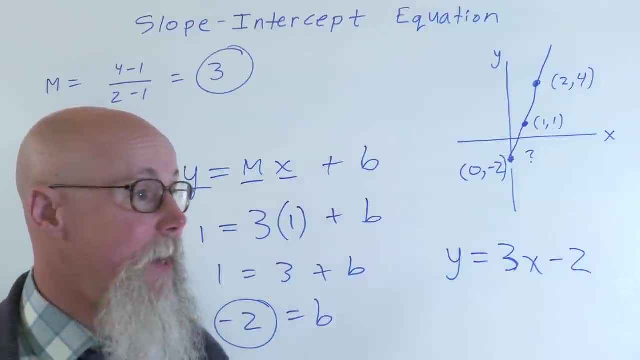 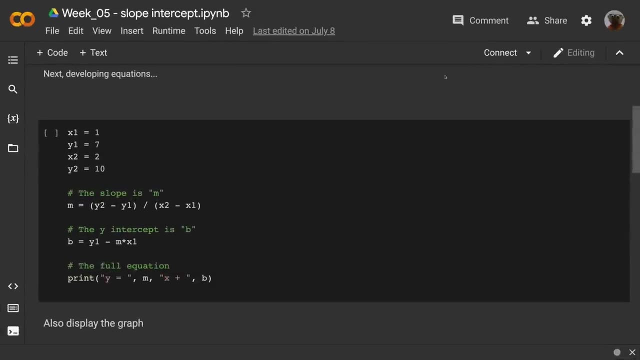 slope. I'm going to figure out the full equation. So we're going to look at how to take two points and develop a slope intercept equation. So now we're going to put it all together and develop the equations. So, like before, we're going to define. 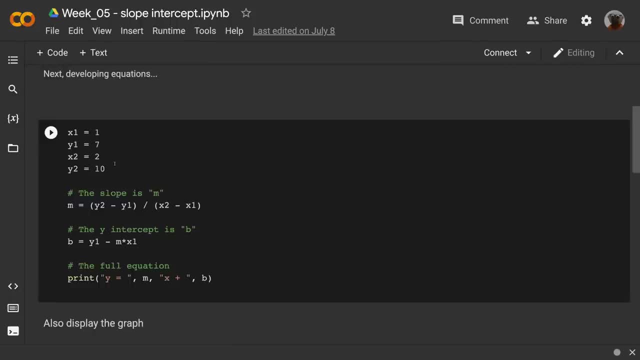 our x1, y1, x2, y2 from two different points And we're going to calculate the slope, which now we're going to call m. That's been the go-to variable for slope m, for how much the line moves. 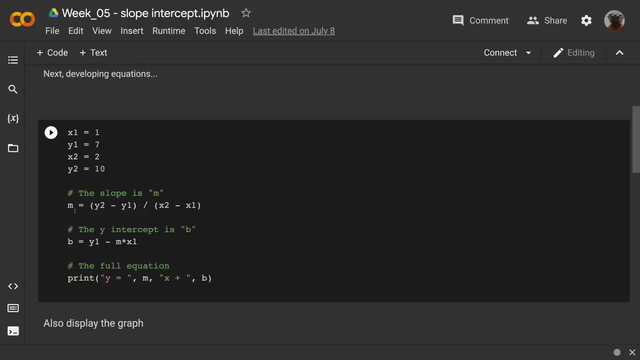 So same formula, but now it's going to be: m equals y2 minus y1, divided by x2 minus x1.. Then I'm going to define the y-interference, which is b, and that's because that's where we begin. 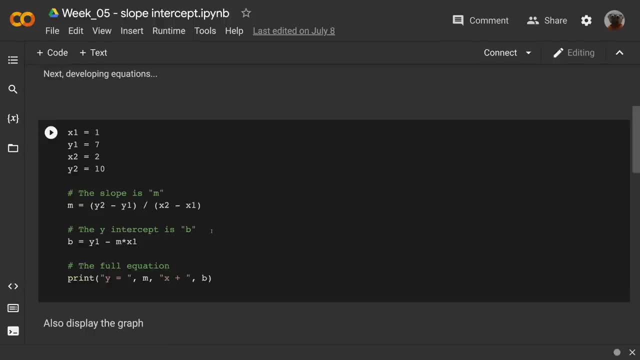 Many things happen in the first quadrant, where everything's positive. so we begin on the y-axis, somewhere where x is 0. So we'll connect this with the algebra that we looked at. How do I, if I know a point and an x, so an x y. 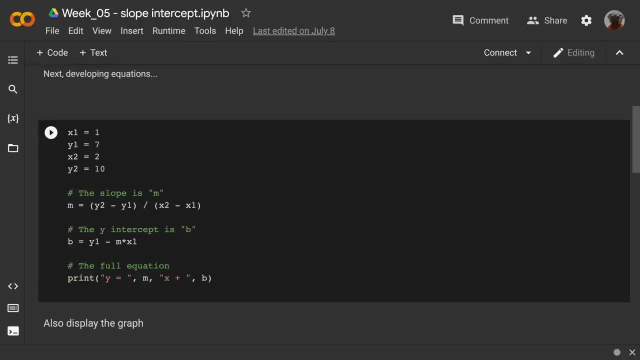 value and a slope. how can I solve for b? A couple steps of algebra. so then b is, you know, y1 minus m times x1.. Now I have m and b, solve. print out the equation. So this will just print out the equation. 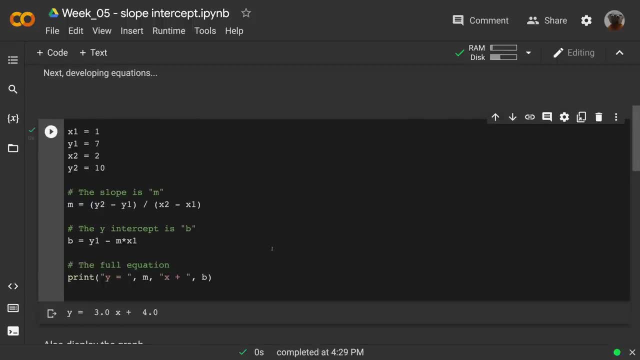 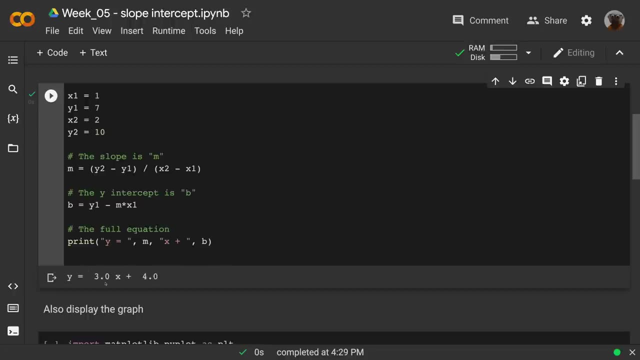 and we'll see that it'll display nice: y equals 3x plus 4, and I still it will still by default give it as a float variable, so 3.0.. It's not worth trying to cast it as integers, because this: 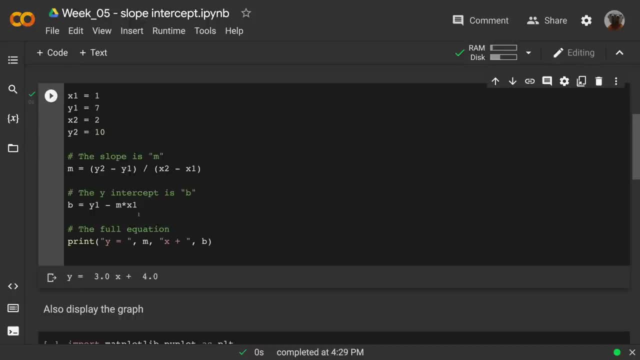 is going to work for any number, and then that way it does not have to be an integer to make this work. So there we go, Knowing these, calculate the slope, calculate the intercept, and then put it all together in the formula. So then, 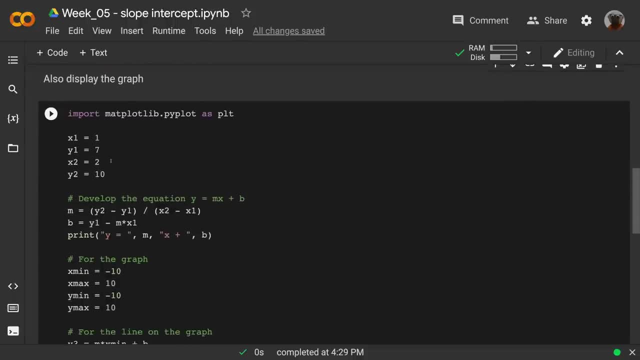 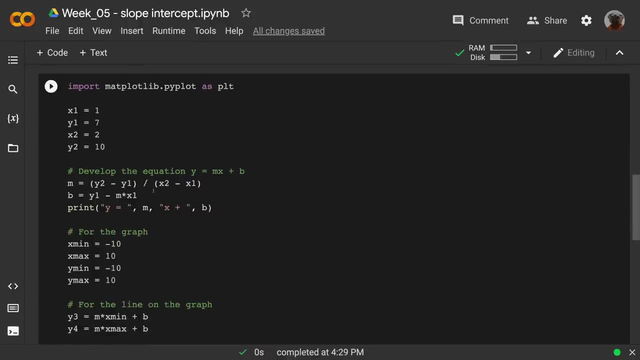 let's graph it: Same thing here, defining my x and y points, and I just kept these same points here. So develop the equation: m equals, b equals, just because we want to print it out, so that we're going to print out the full equation. 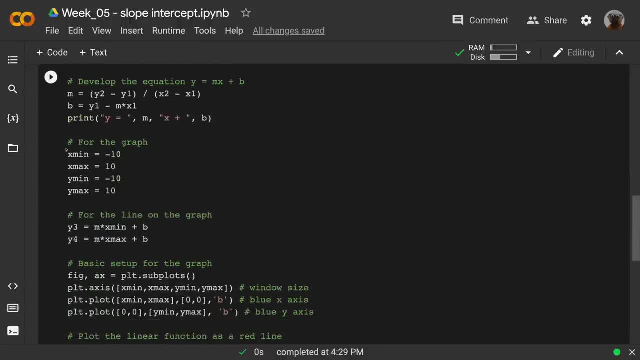 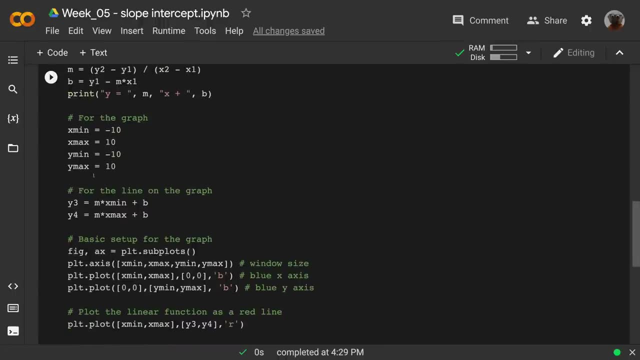 and now we're going to go back to the graph that we were doing before: Define our x min, x max. Now, how do I want to display this line? I can graph. I can find two other points, So I'm going to take the x minimum. 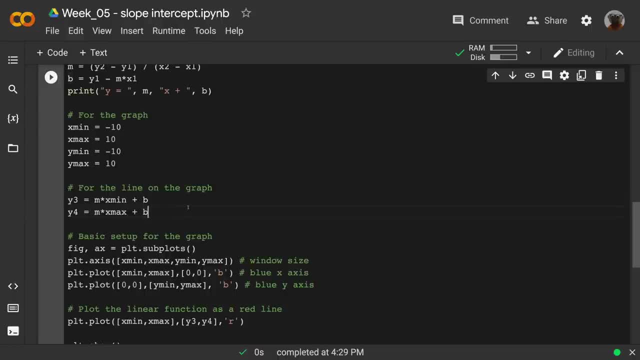 so we see here in the first line y3, I'm going to take the x minimum and I'm going to convert that times m plus b. that's going to be my y value, and then I'm going to take the x maximum. 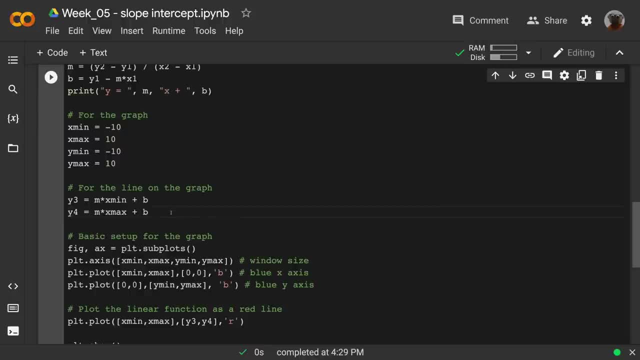 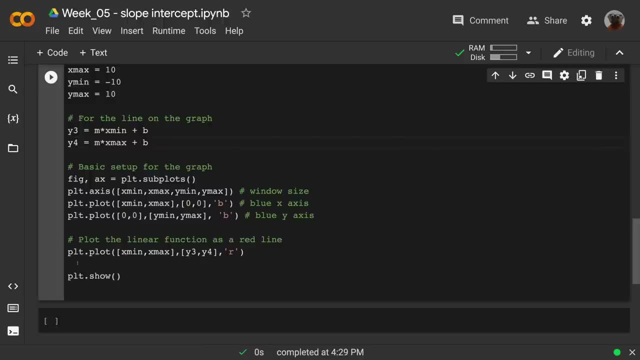 times m plus b. that's going to be my other y value. So now I have these other two points, Basic setup for the graph, same as we were doing before and we have now. I'm going to plot that line, plot dot. 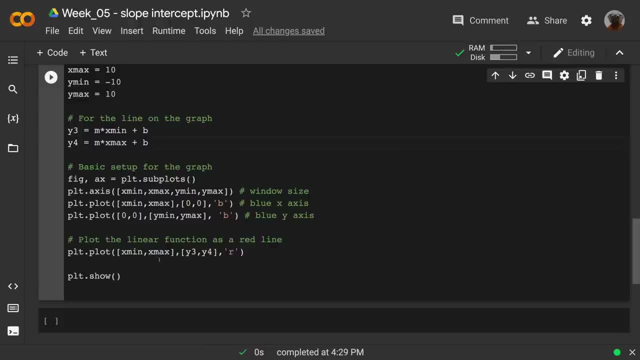 plt, dot plot and my x values are going to be x min, x max and my y values will be these new y values And I'm going to plot this as a red line. So if I put an o in here, 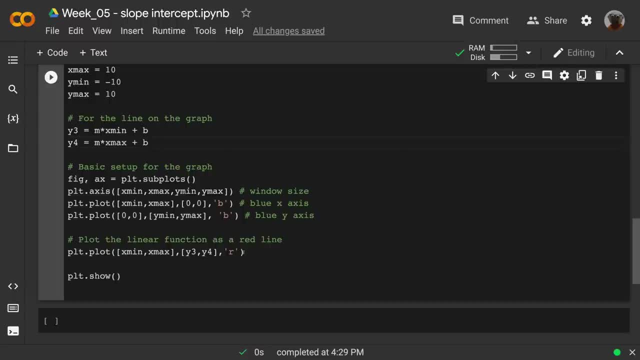 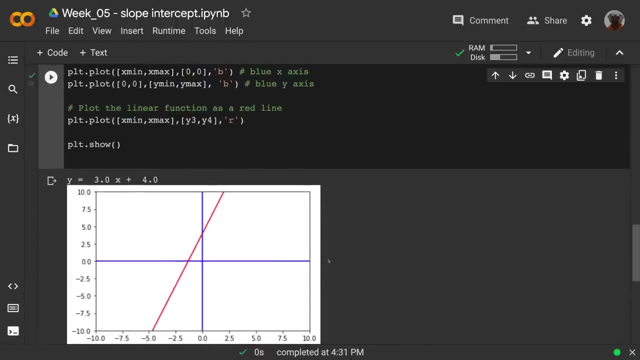 that would put these as two separate red points. but just r makes it a red line. And now when we run this, there we go, We calculate the equation and we graph the line. Good times, So I can change anything else. 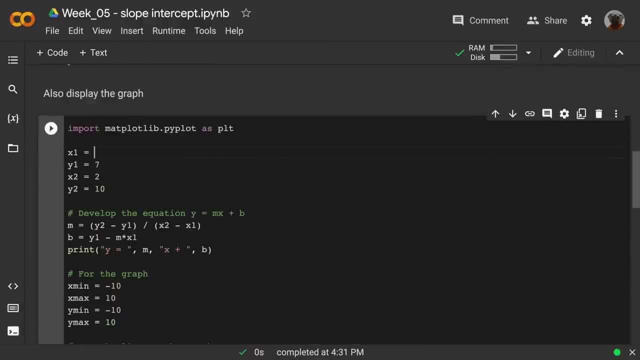 I can have any other two points. There we go, There we go, Two, three. and if I kept the same x value, we know this, actually some of this would break, but it might still graph it. but we know that that's not a function. 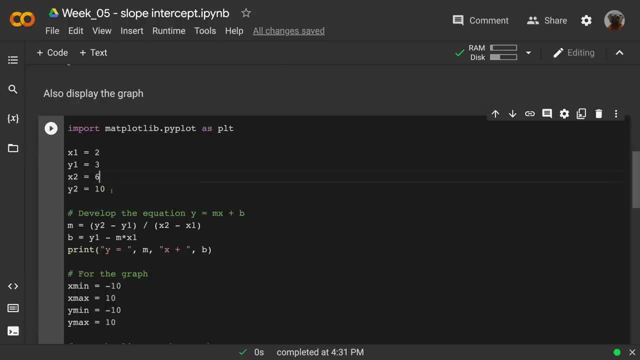 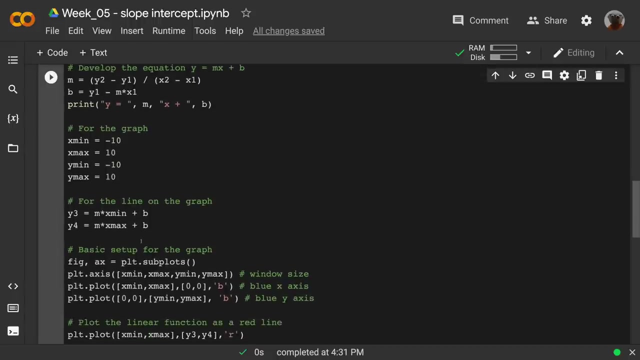 There. So there we go, Six, and I'll make this one eight, Just to show that we can just change these and all the rest of this will work. Solve for m and b, get our equation, plot them here and. 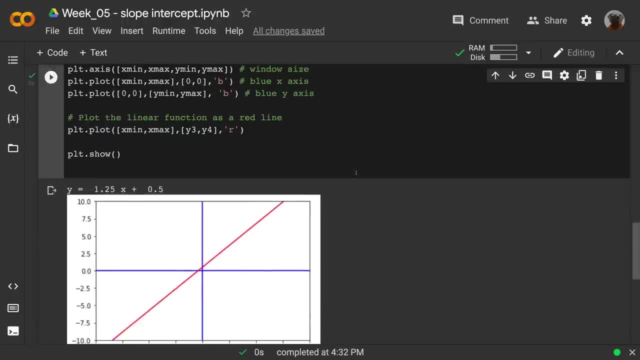 when I run it. there we go, So 1.25x plus 0.5, and we see that it must cross the y-axis at 0.5, and then that slope up 1.25 over 1.. 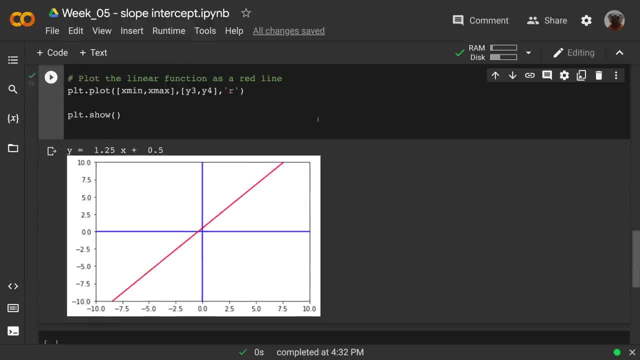 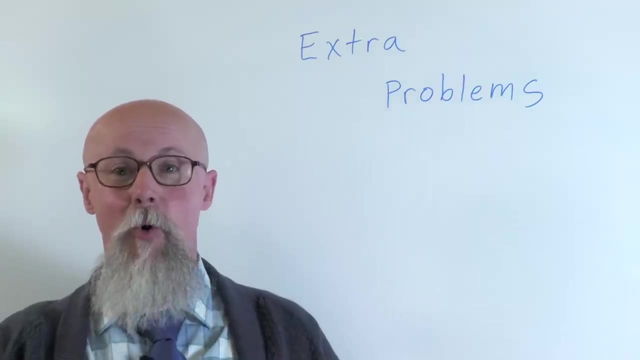 There we go, Alright, so now we can graph and do whatever you want with the two points you find. Now that we've worked through the core skills in this unit, let's look through some extra problems, and I'm going to work through extra problems. 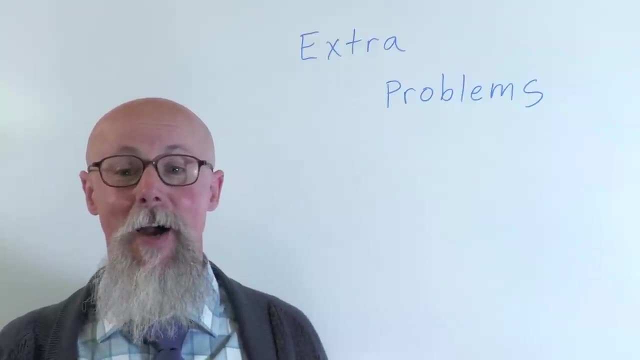 using the Colab notebook so you can see how you can apply these resources that you're building and use these to solve problems that might come up in a textbook or in day-to-day life. So we're going to go through some more extra problems here. 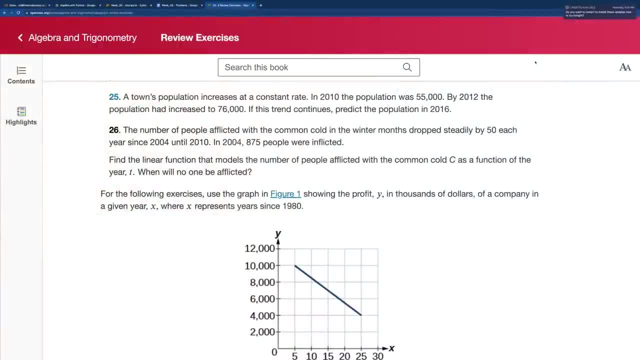 So we're looking at how we can apply some of the things that we've been doing to real life situations and use this information to predict things, to figure out some trends and real life or things that show up in a textbook that hopefully are realistic. 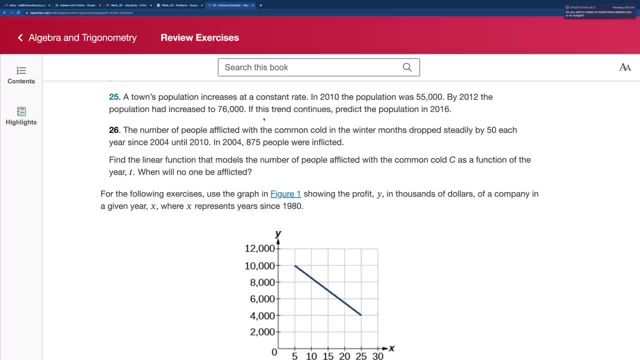 enough. So let's take a look at some examples here and we'll work through these. So, if we look at 25,, a town's population increased at a constant rate In 2010, the population was 55,000.. By 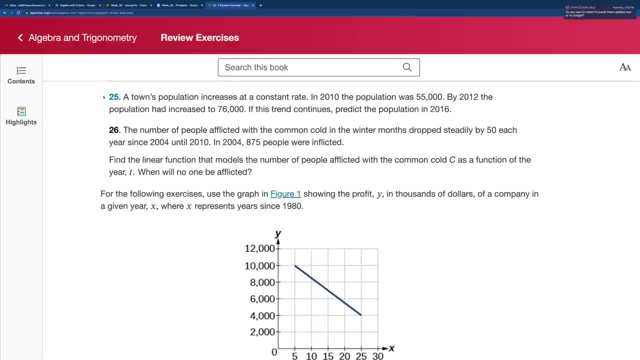 2012,, the population had increased to 76,000.. If this trend continues, predict the population in 2016.. So we want to notice that these are two x-y coordinates: time and population And time, if you have it. 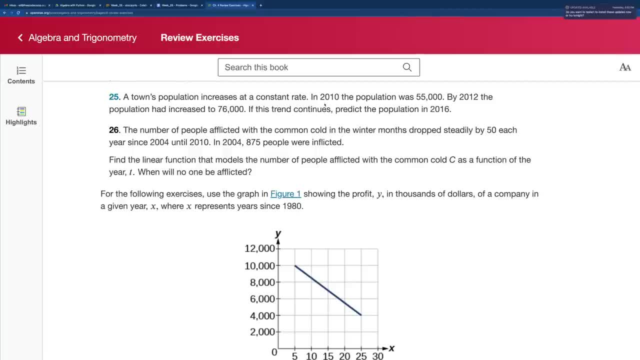 it's going to be on the x-axis Almost all the time. So, if we look at this, so 2010, 55,000.. 2016, 76,000.. Or 2012, 76,000.. 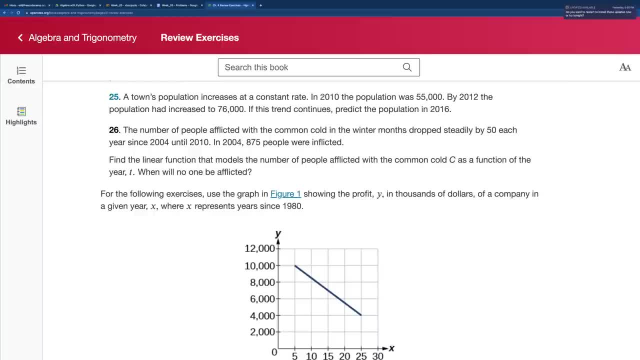 So when we do this, we have- I could make 2010- the x value, but I could say, hey, this is the beginning of this situation. I'll call it time zero. So in time zero and 55,000, these are nice, even thousands. so. 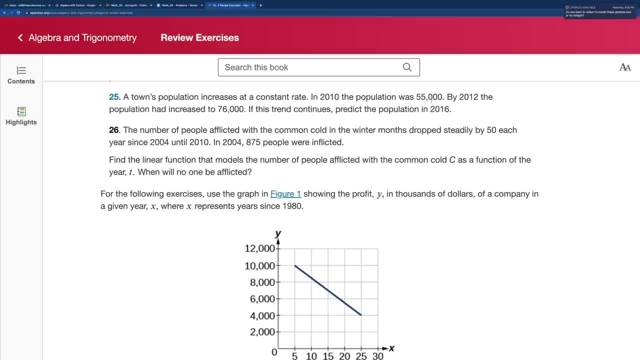 I just might call it 55. So time zero, the population is 55, and 2012 is when we have the next year, So that's two years later. So two and then 76. So we want to take notice that. 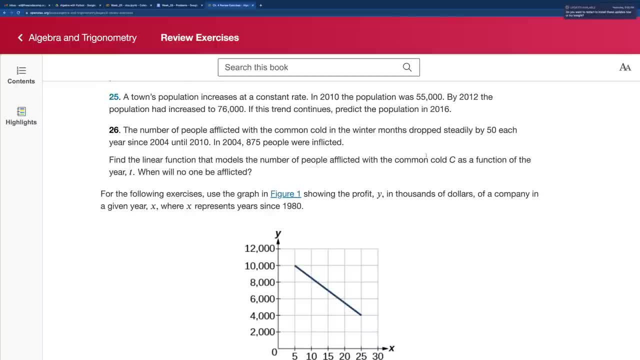 we're recognizing these as x-y coordinates that we can put on a graph And we're going to use that. we're going to predict in 2016.. So let's take a look at how we would do that Now. hopefully you've. 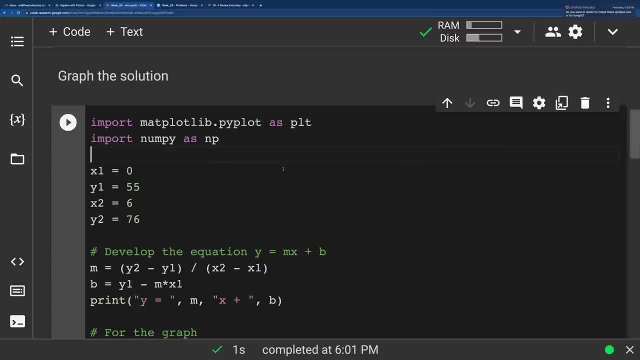 already been putting together some things that you know you can use to graph. you know your colab notebooks, so that you would already have this, something like this, set up. You know graph. You've already done the imports. 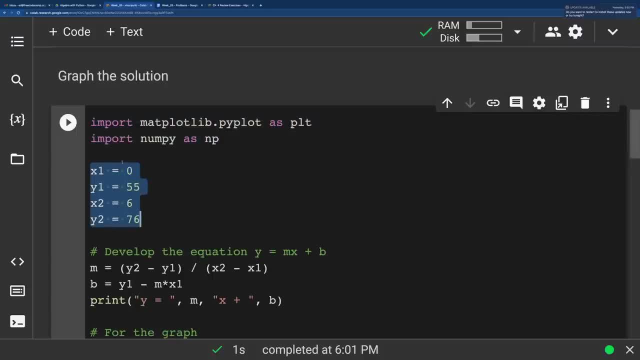 This is the only thing that we're changing. Remember this for the two points. and then we're going to calculate the slope and the intercept and everything. So x1, 0, y1 is 55, x2, I would want that. 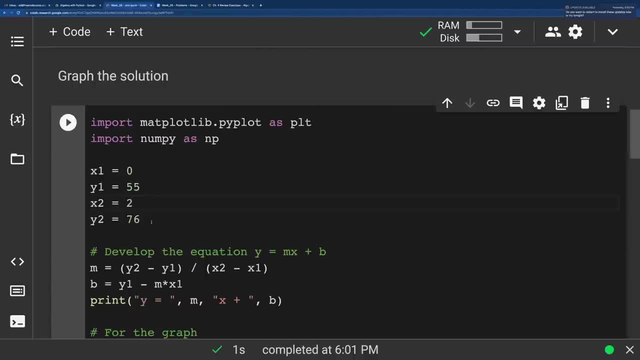 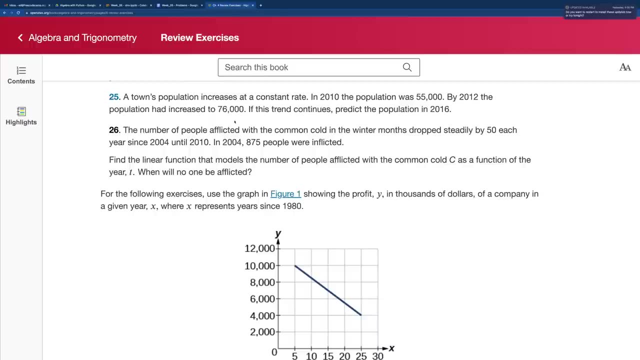 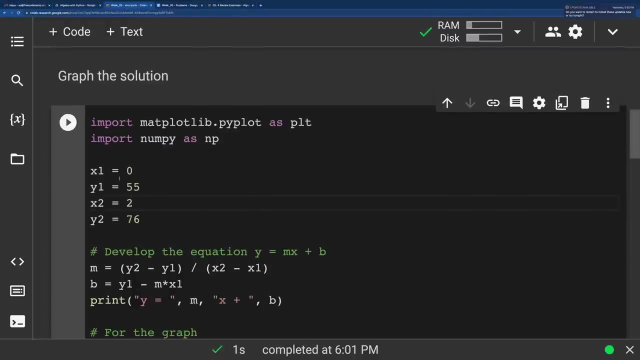 to be 2, and y2 is 76. So you see that that matches up 0,, 55,, 20,, 12,, 76,000.. And these? this would then be the only thing you needed to change. 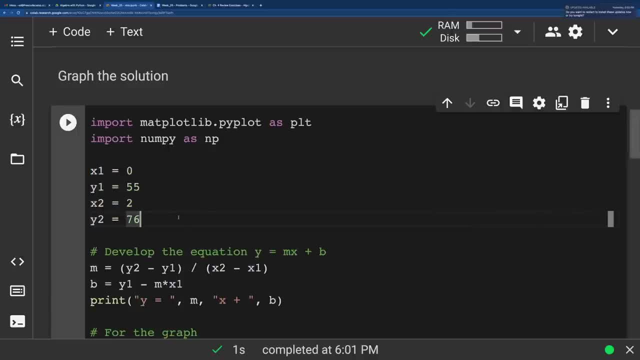 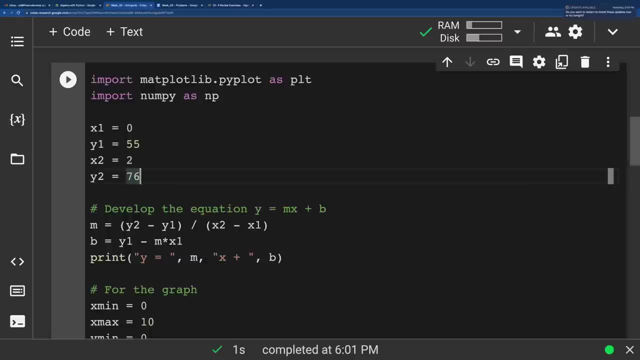 is your two points, because all the rest of this you'd have. this you know already, set up, Develop the equation. So you know, we're going to calculate the slope, We're going to use that to calculate the y-intercept. 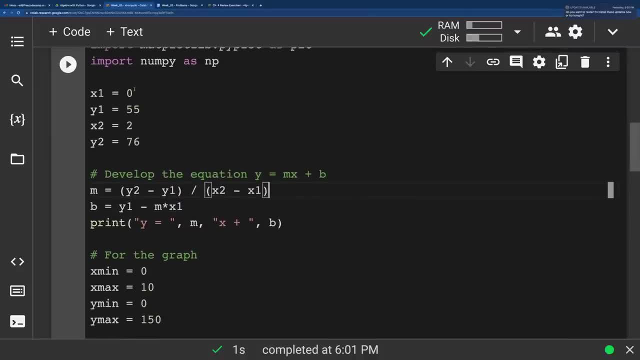 Now we happen to know, because we have: x1 is 0, so we know that the y-intercept is going to be 55.. But that's okay, We're going to print out the equation and then our classic graph Now. 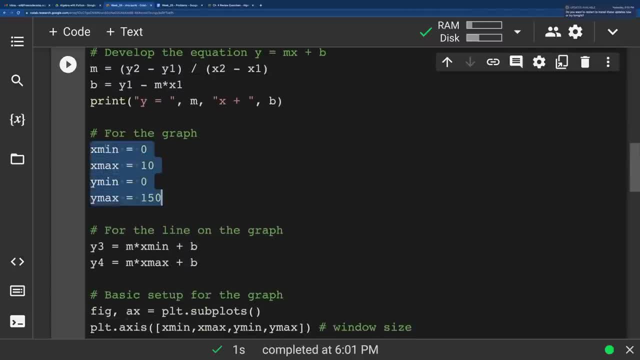 I would normally have this set at: you know, negative, x-min negative 10, x-max 10, y-minimum also negative 10, y-maximum 10.. So this is the other thing that we would change, because 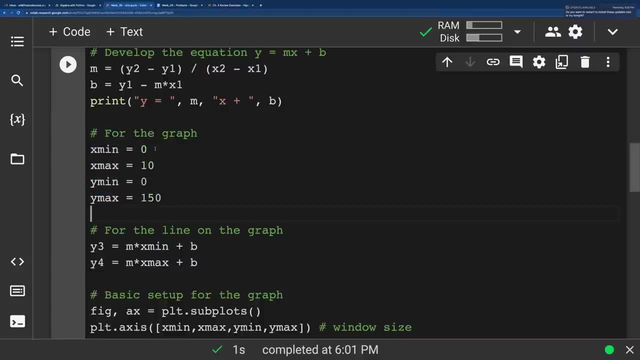 we look at this graph and an x-minimum of negative 10, so in time that would be 10 years ago, but you know we're not going to worry about going in the past and making that negative 10.. 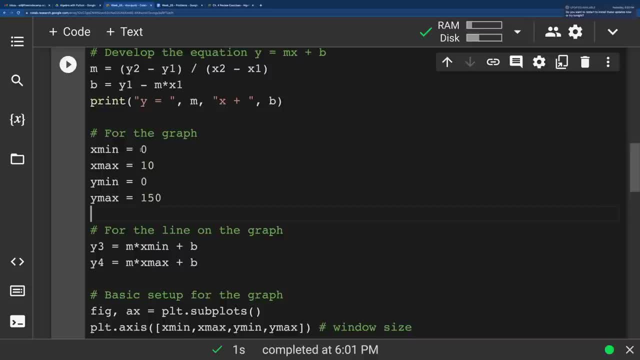 So I'll just keep it at 0, and we can, you know, look at it from there. Then x-maximum 10, we can keep that. That's probably just as good. You know, we're looking at the most. 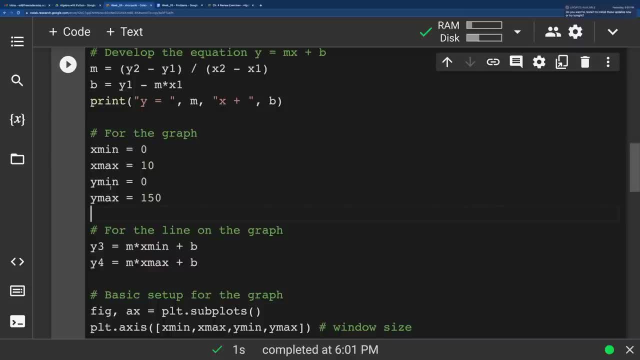 6 years for this situation and y-minimum, I'll also make that 0. Actually, because y is population, so y-minimum being less than 0 would just be weird Negative population. they're not going to be in the upside down or anything. 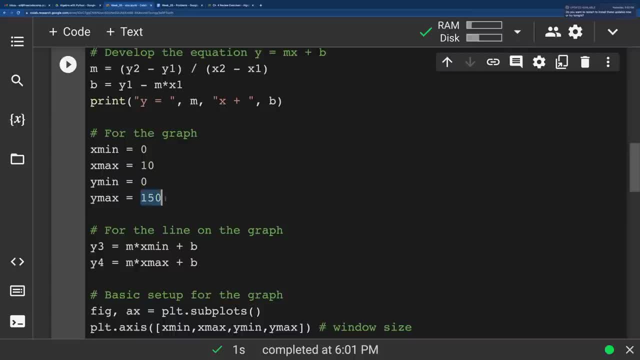 Alright, or y-maximum, and I picked 150 because we already started 55, and then we're going to 76, and we're predicting a few years in the future, so I wanted to go up a little bit. 100 didn't seem like enough. so 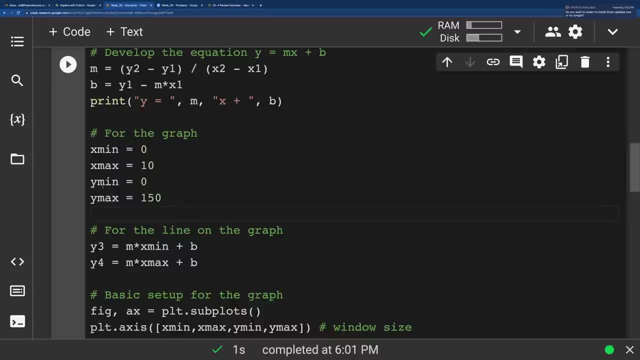 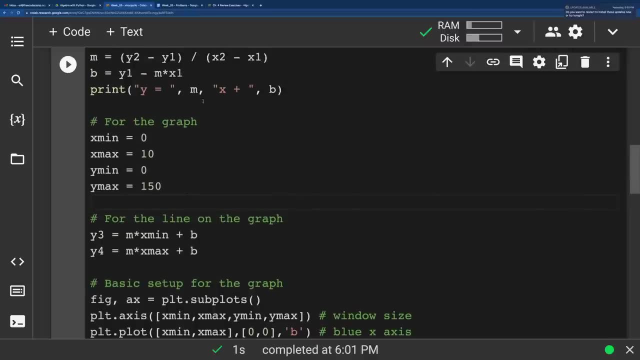 we could always change these, So all we need to do is change these and notice all the other things for the line that we're going to graph. So notice, even though I'm printing out this line, I'm still just using these. 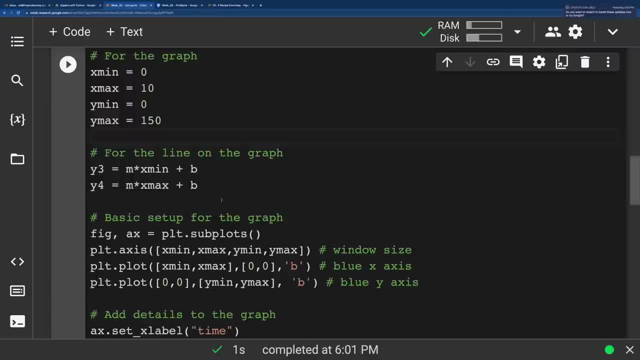 x-min and max and then two more y-values to calculate this line, and we're just doing the line that way. There's other ways to do this, but we can keep this for how we're going to display this line. This works for. 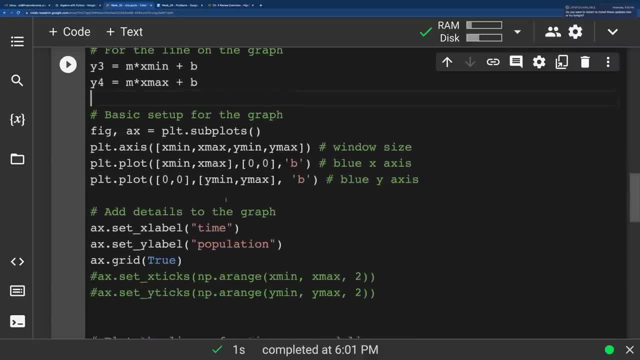 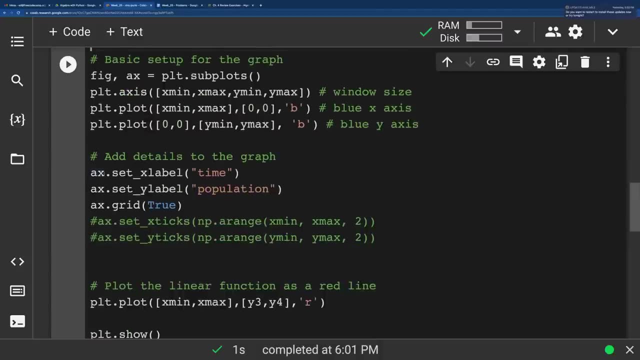 linear equations And we still keep our basic setup. Now here's where we'll also add the details. so again, hopefully you have these and you could also comment these out and then use them as needed, Like I have these commented out about setting. 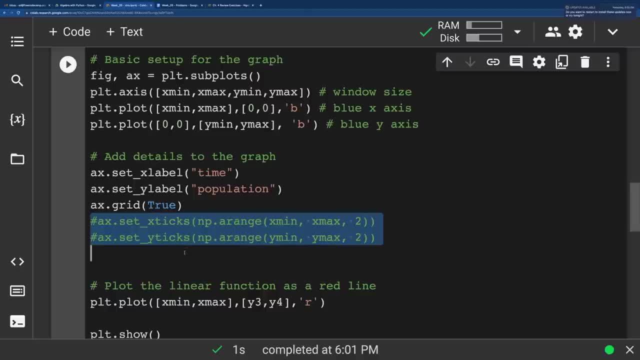 the x-ticks and the y-ticks. We'll see if we need to. We'll see if we need to change that And you might have the default x-label as x-values or y-label as y-values, but we can change these here. 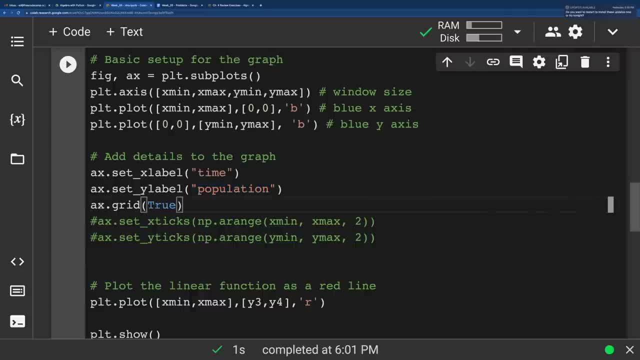 time and population, And I like seeing the grid, especially for this situation, so I'm going to put that in as true. So we have these details that you could have your setup and have these all commented out. All you need to do is uncomment. 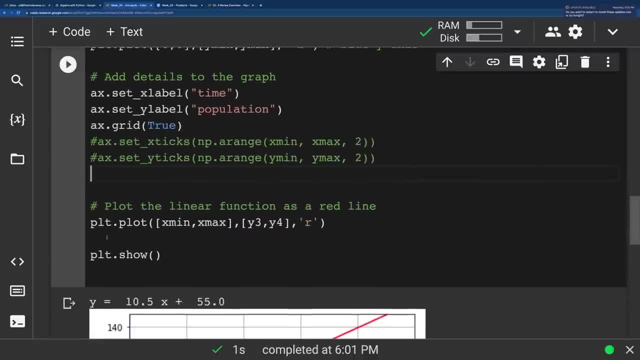 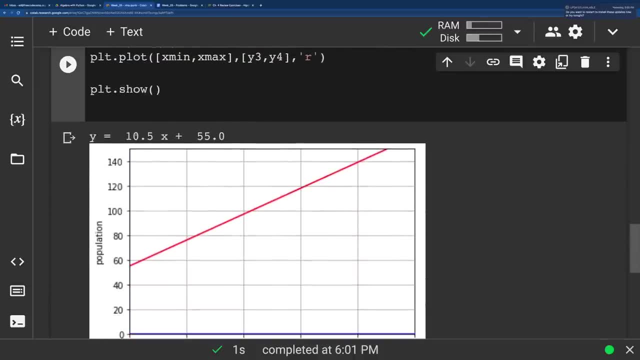 them as needed. And then there we go. we're going to plot this linear function and then here's what it looks like when we run it. So we figured out the equation. so it's going to be there it is. 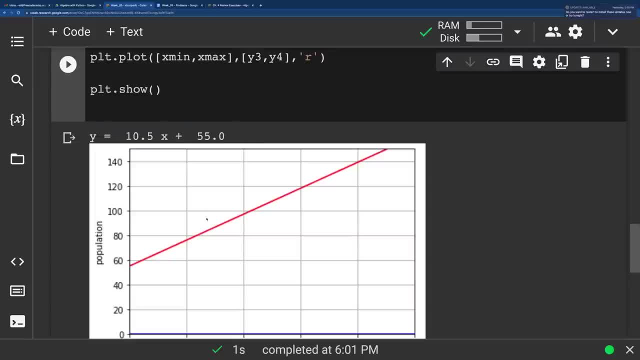 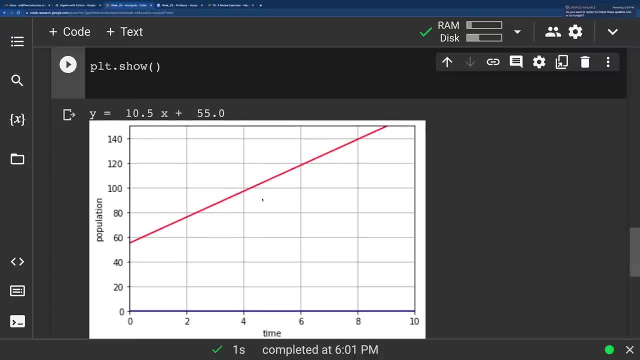 10.5x plus 55.. So we see this trend and we see it starts at 55, increasing about 10,500 every year. So year 2, we see, yeah, I'll estimate that as 76.. 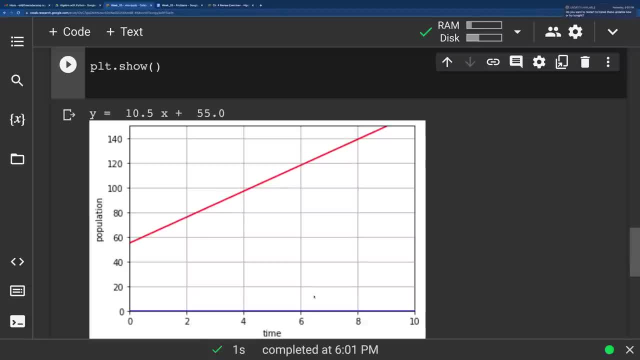 Year 4, and then year 6,. this is what we want. Now this might not be exactly 120.. We could plug that in and see, because now we have the equation, You know what is the value at 6 years. 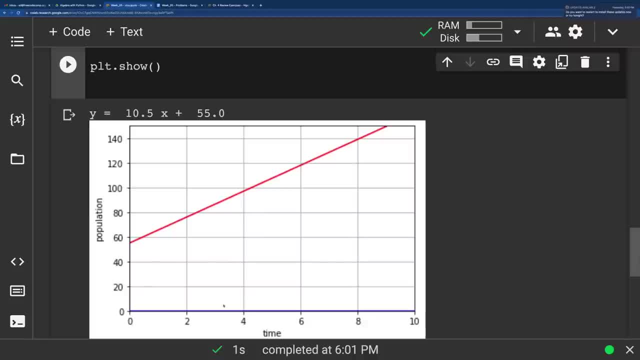 But also, this is enough, and that's why I didn't worry about changing the tick marks, because the default that it gave us, I think that actually ends up being pretty good. So there we go. As a good enough estimate, I would say: 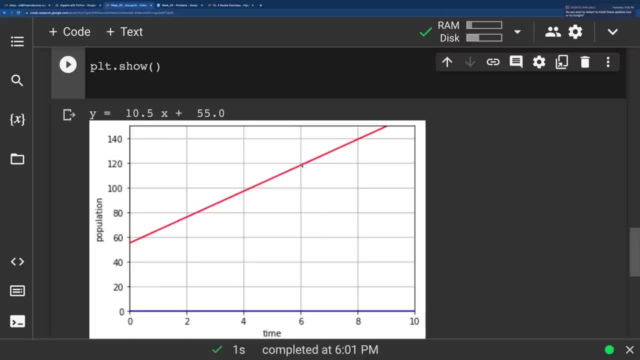 120,000.. For you know population estimates, you know the fact that it might be, you know 119,500 or something like that. you know our rough estimate is going to be 120,000, and that works. So you see. 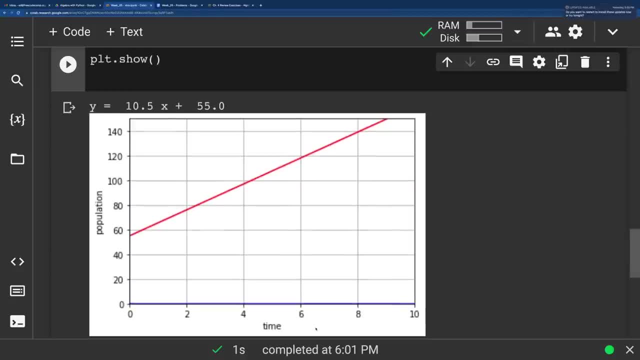 and then we have our dice labels, time and population. the grid marks help. So this is how we want to do this. We can, you know, we can- set up this equation and see the graph, and that helps us answer all these questions. 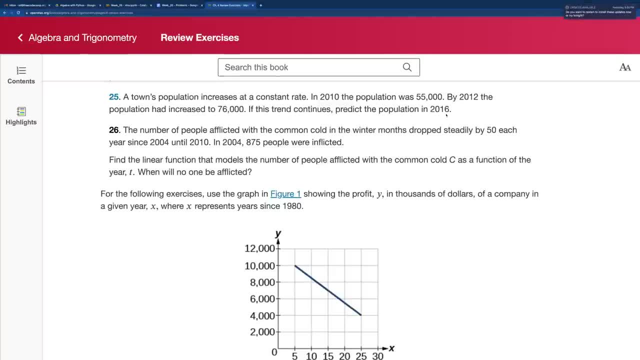 There we go, We see the trend and we can predict the population in 2016.. Oh, it's about 120,000.. Alright, now here's another one. The number of people afflicted with the common cold dropped steadily by 50 each year. 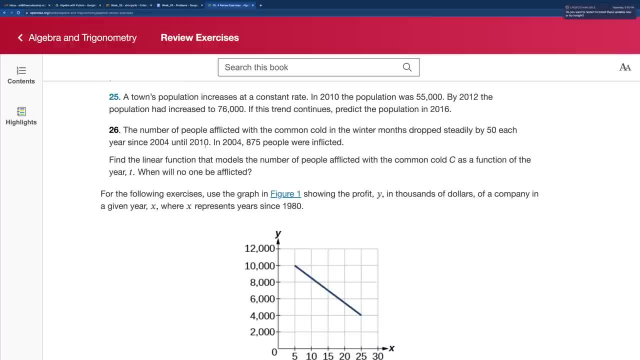 since 2004 until 2010.. Okay, so we're looking at our key words here. So dropped steadily, then we're talking about a subtraction And then I'll make times: zero: 2004,. since 2004. 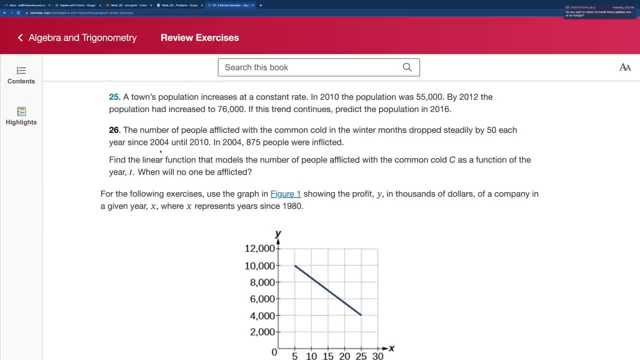 is the first year we mention this Now also a lot of these in real life. yes, they wouldn't be perfectly linear, but a lot of times that linear trend gives us a decent enough approximation, and that's the idea for some of these. 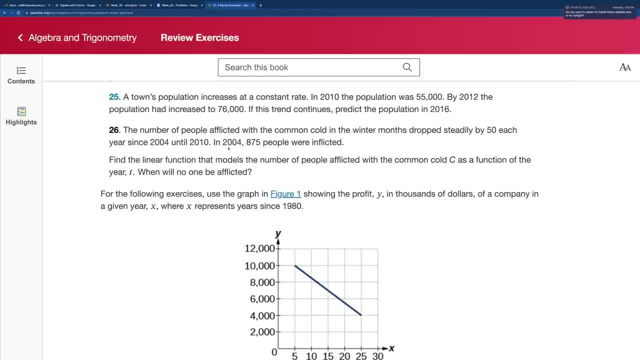 It's enough of a prediction. So now we have in 2004,, 875 people were inflicted And notice, even with the comma there you can definitely see there's your xy value Year and then afflicted, And then in 2010,. 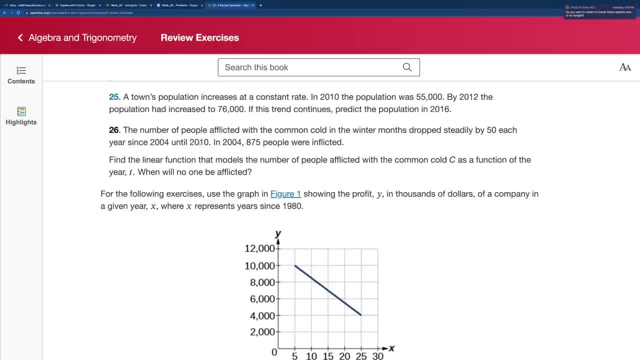 it keeps dropping. So one of the things that we can do here- well, this is find the linear function. So one of the things we can do is I can make 2004 times zero, And then that's 875.. 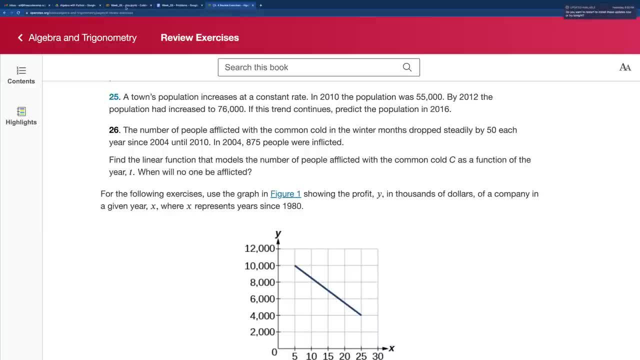 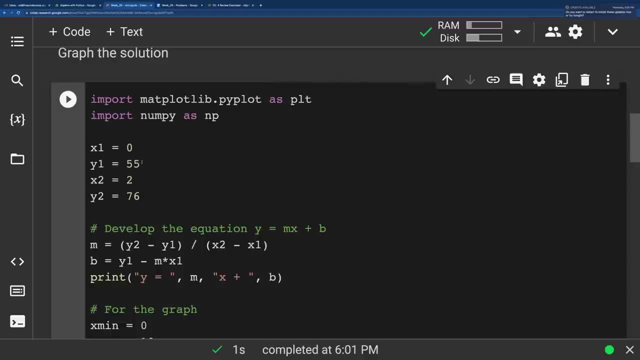 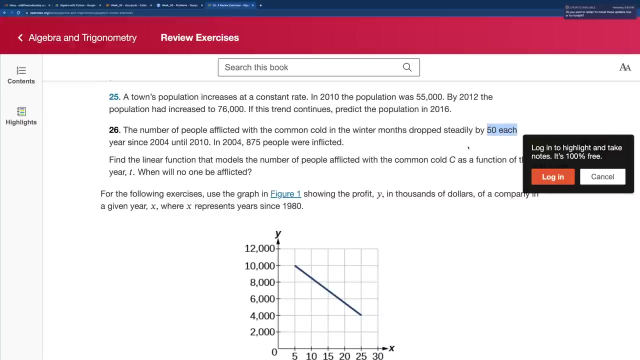 So if we take a look at this 2004,, I'll make that times zero, And then this one, I'm gonna make 875.. Alright, so now, if it drops steadily by 50 each year, all we have to do? 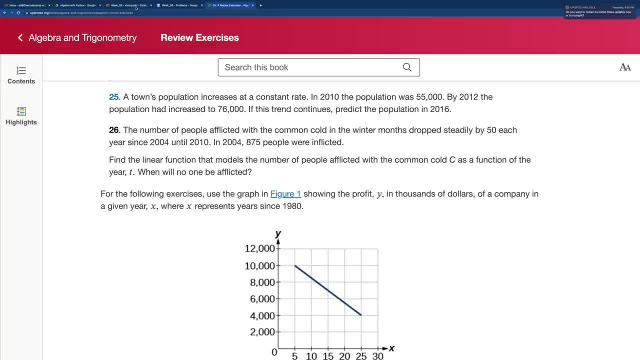 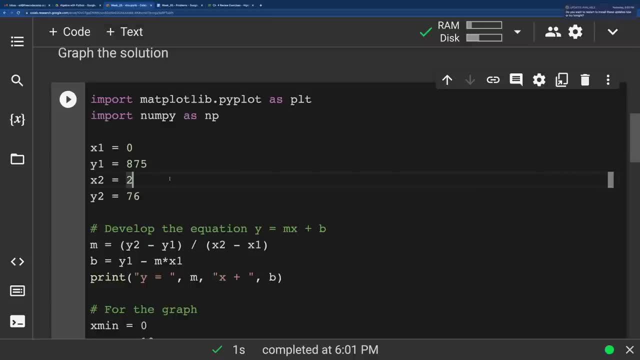 is. we just need one more point. if this is linear, So we can just do the subtract- you can do the subtraction in your head here- Then if we have year one, then it drops 50.. So then that's gonna be 825. 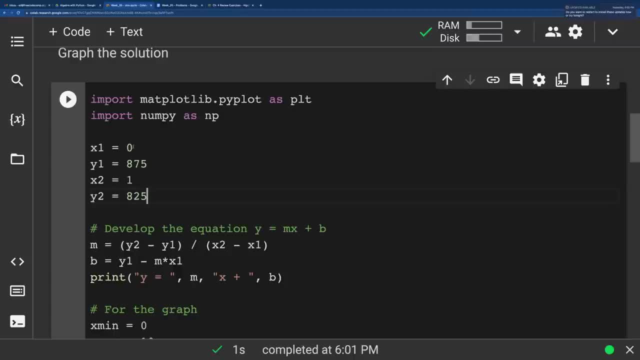 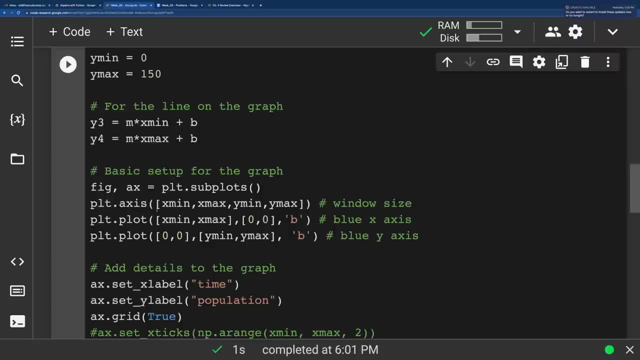 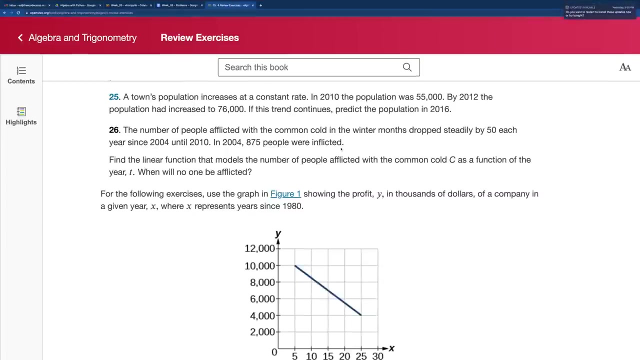 And you see, that's all. we need two points and we'll be able to do everything else: Calculate the slope, calculate the intercept and display the equation. I might even well now the time and population won't mean anything. 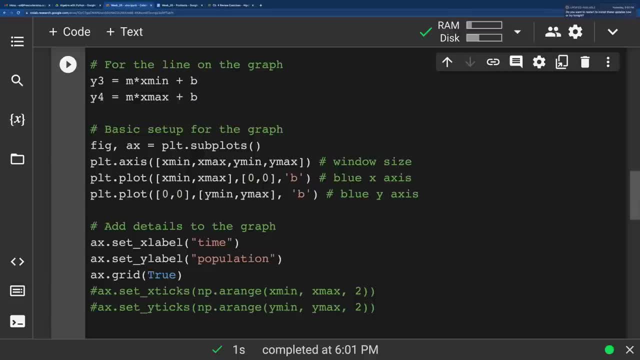 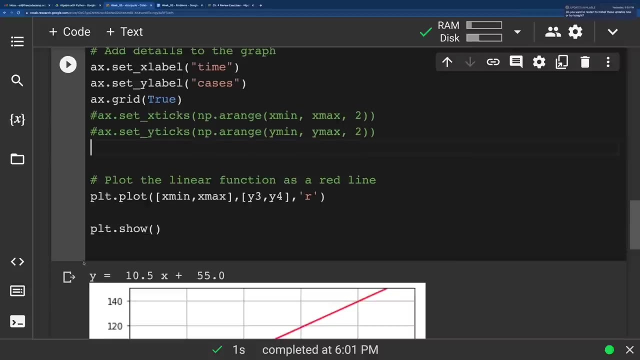 So you know number of people afflicted, you know how. about cases, Number of cases of the flu. There we go. So there we go, Time cases and you can hit control or you can hit shift enter. 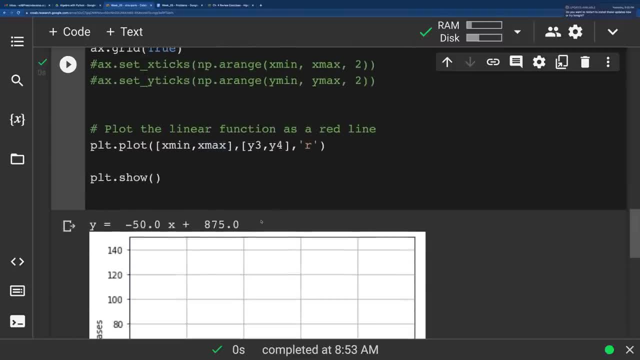 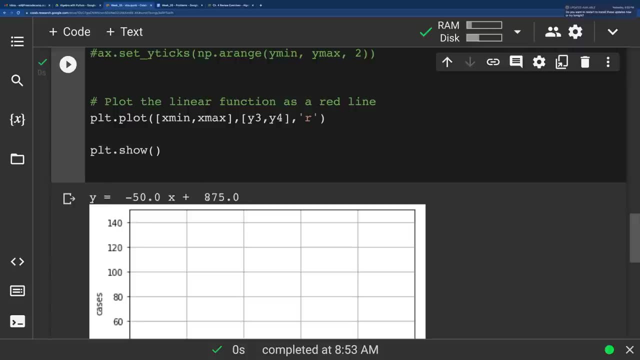 or click this And we see this trend. negative 50, was still in the y equals mx plus b. negative 50x plus 875. And a lot of times you would see this, they'd put the 875 first. 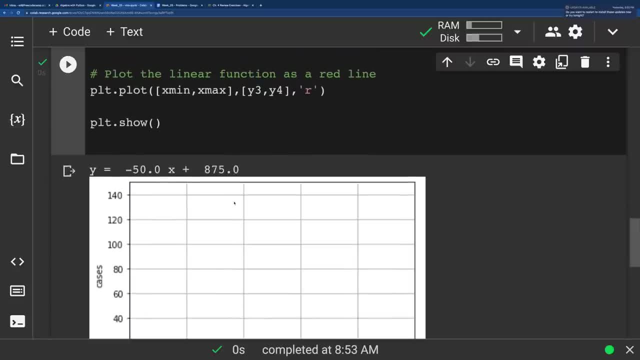 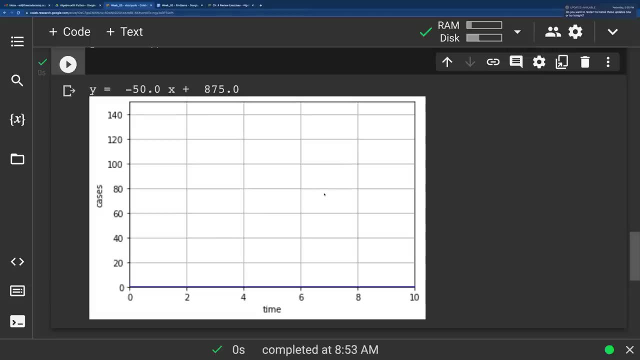 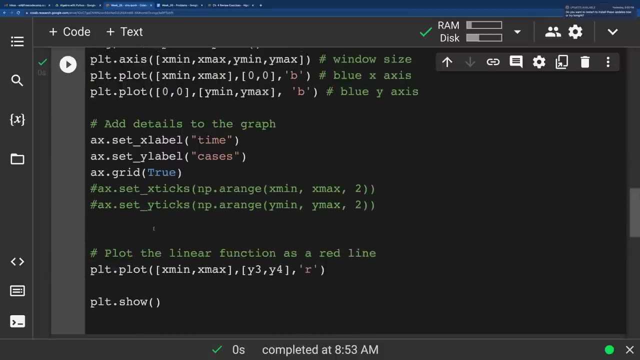 and then subtract. but that's okay. Now also this: notice that you know my xy axis. I'm not going to show anything. Why? Because it started at 875, and you see, 140 doesn't cut it. 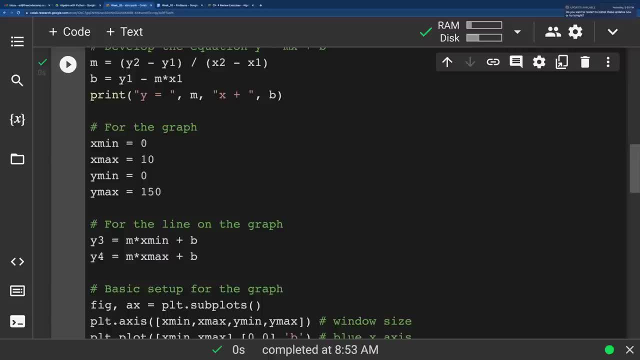 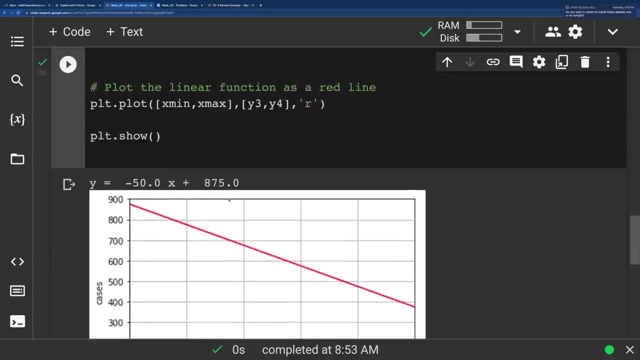 So we have to go to x minimum and maximum, that's fine, y minimum, that's fine, but y maximum it can't be 150, maybe I'll call it like 900.. So now we can see the graph. 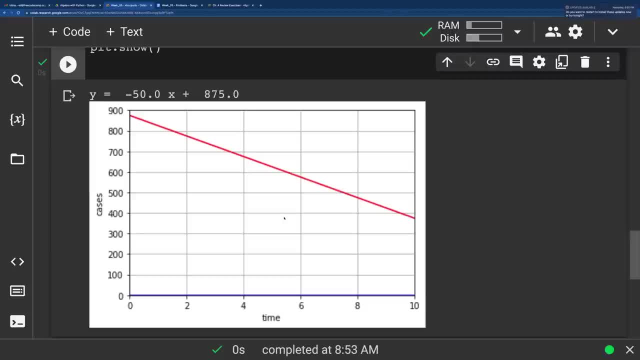 And sometimes you know, you graph it and you say, well, why didn't it show up? and then you look and see, oh, it's the window. Well, I'm out of bounds here. So there's 875, and we see this downward. 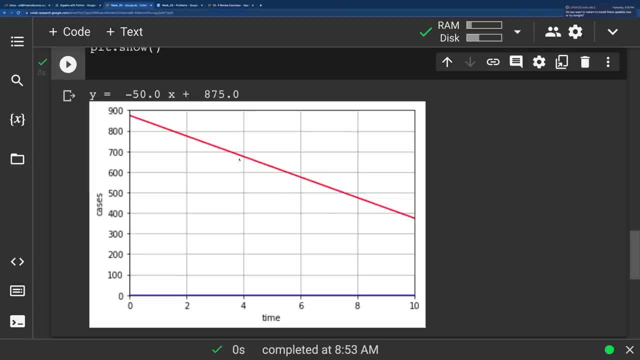 trend. So there we go, And we can use this to predict, you know, in any year. Now there's other ways to get the exact amount We can you know for any year. we can actually plug in that. 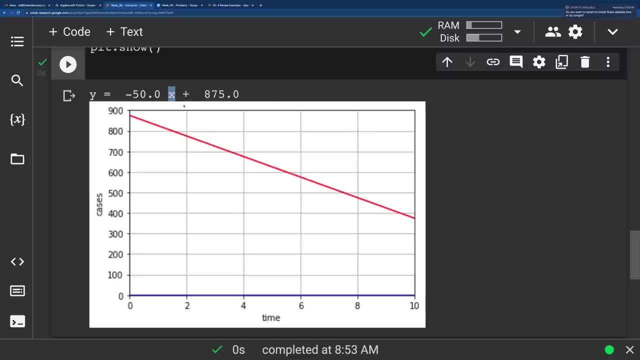 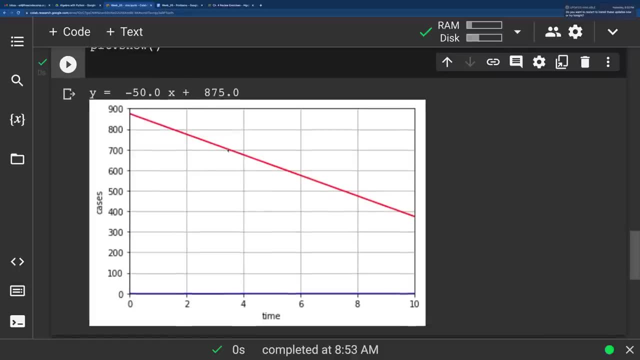 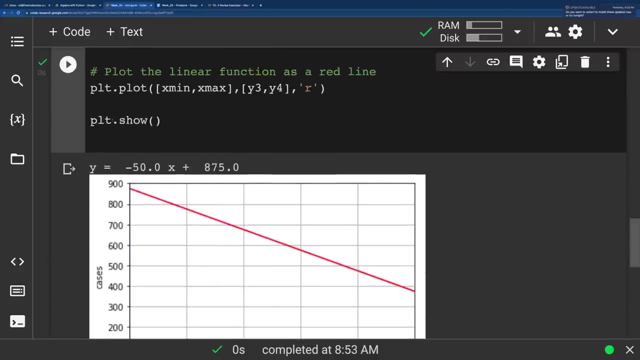 x value and then solve. so that works And remember that even works within a print statement. So if we have So the interesting thing is this plotshow that needs to be last. so if I do another print statement, I would do it. 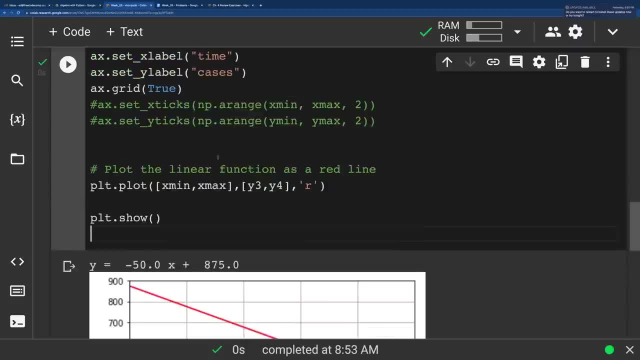 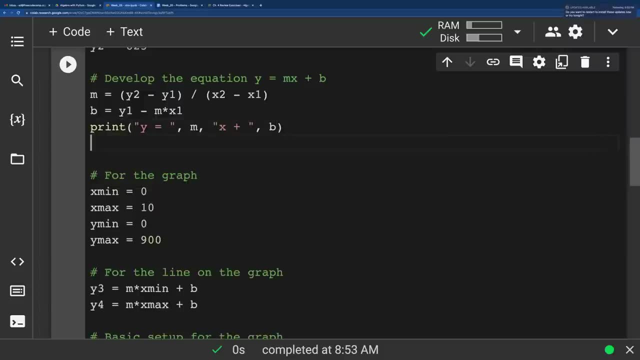 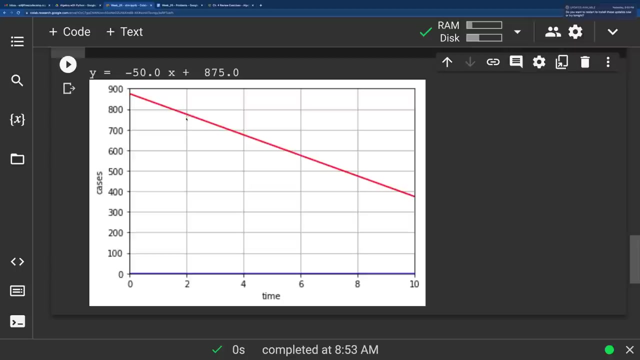 later. But I could, right under here- you know the same place where I print this- I could print. So what if the question was how many? you know what's? how many people had the flu? We might say, oh, look at this, two years. 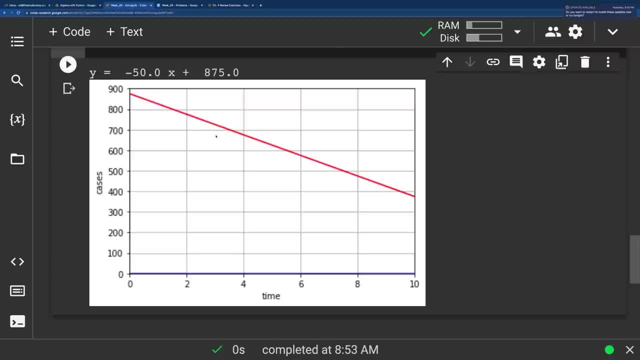 later. you know we had the, Now we can do the subtraction, so let's say like five years. And you see, given our graph here, you know we see this trend, we can estimate it, but we don't know exactly. 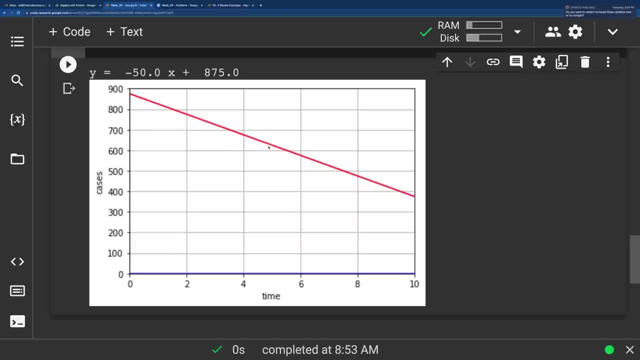 you know it's not detailed enough to see it, So I can say: oh, in about five years how many people were afflicted with the flu, And supposing I want that exact number, So I can go back to this. 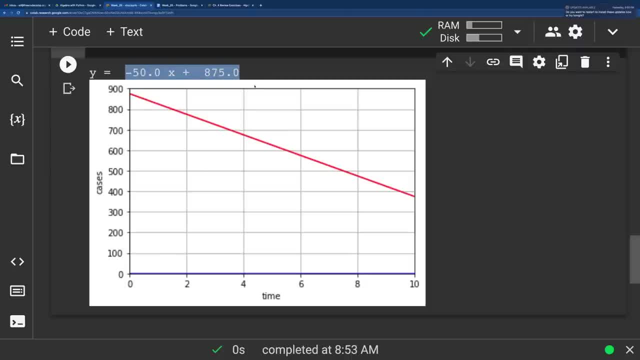 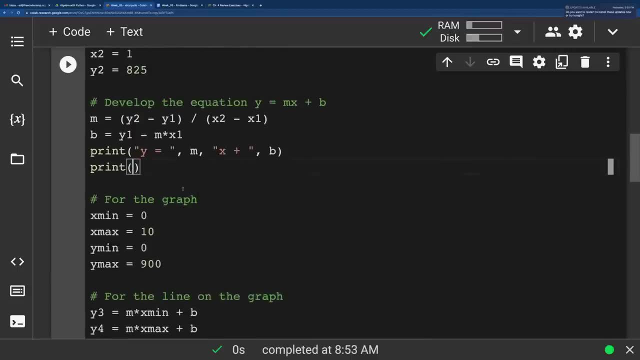 and then x is five. So one of the things you can do is in the print statement you can actually just do the math and you can have like a more elaborate print statement if you want, but we can just do our math here. 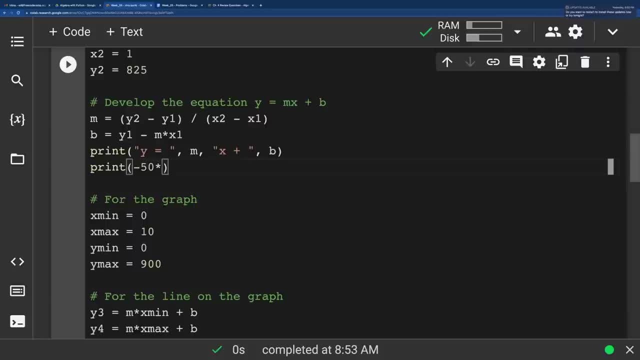 Negative fifty times five plus eight, seventy five. So we see, you know our negative fifty times five plus eight, seventy five, and that would give us the y value. what would be the value? what would be the number of people afflicted after five years? 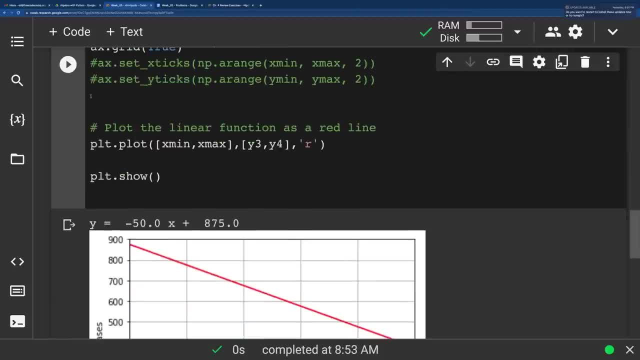 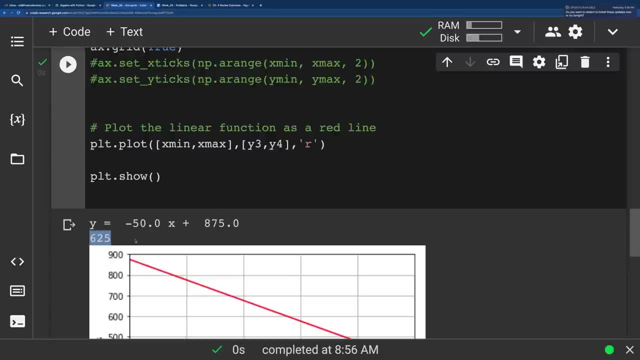 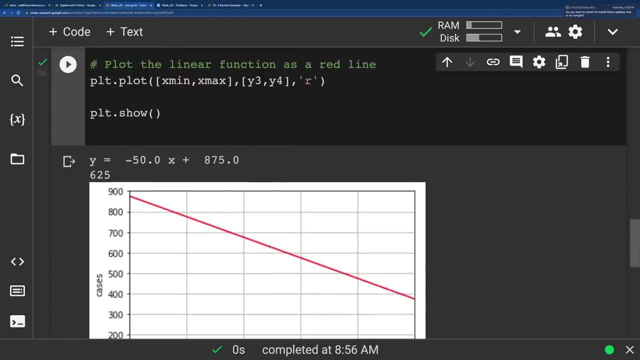 And again, you could have a more elaborate print statement to say something, but since we already know what that question is now, that that's six twenty five, that means something to me when I see it there. So you see, that might be. 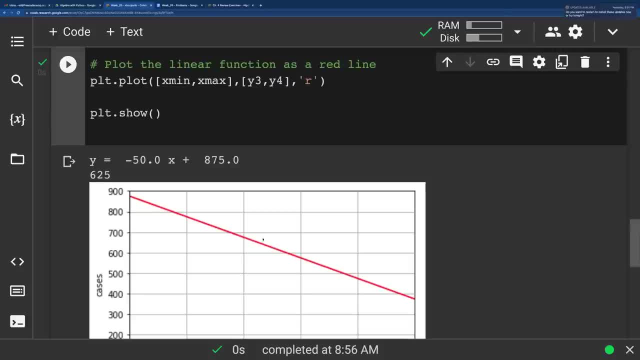 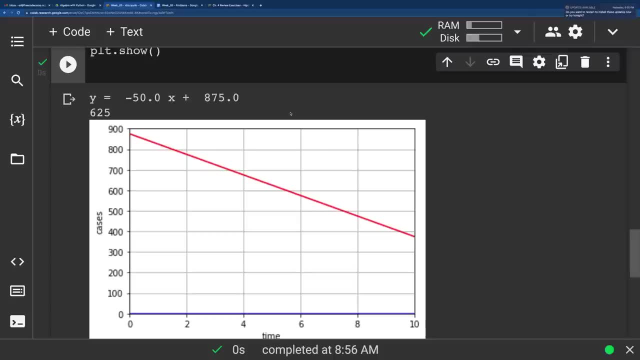 you know, could I estimate it exactly? oh, that's six twenty five. Eh, not necessarily, but I can plug in the number and get it. So we see, you know some different things we can do. see the graph. we can answer. 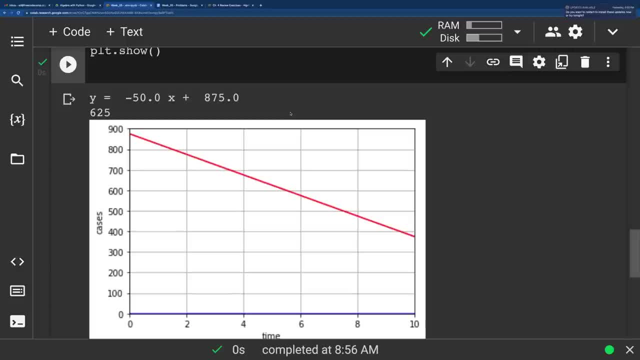 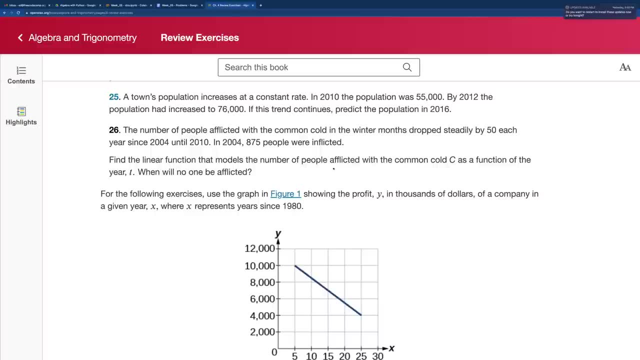 some questions. do some math for you know some specific, some specific questions related to this. Now, alright, alright, linear function. so here's another question: When will no one be afflicted? So we want to know: 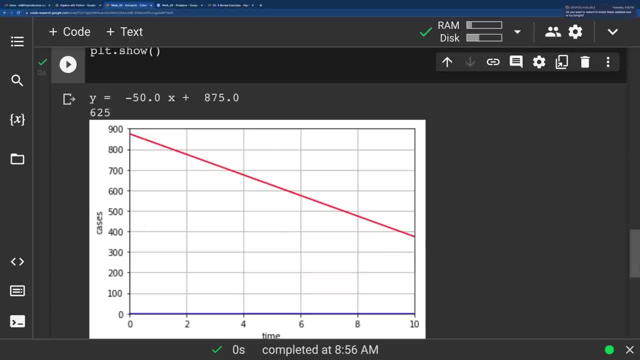 looking at this graph: when is the y value, the number of cases, going to be zero Now rather than now? one of the things- you could expand the graph until it gets to zero. we'll come back and do that in a second. but 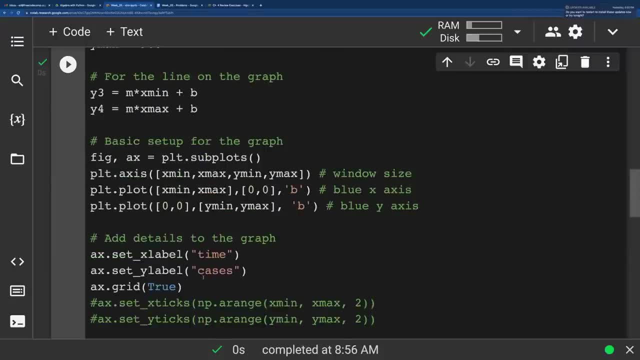 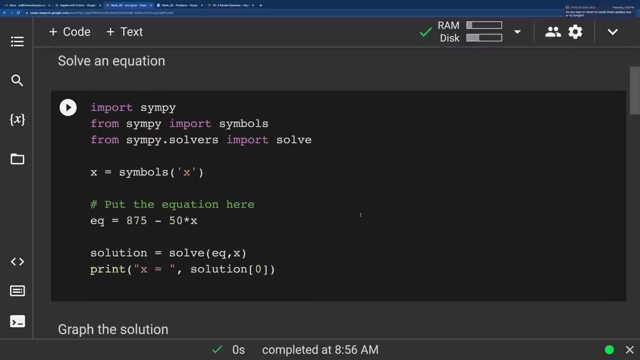 one of the things that we could do is if you already also have your setup to solve an equation, So you know you have this and remember this was the whole setup to solve an equation and print the solution, and so the only 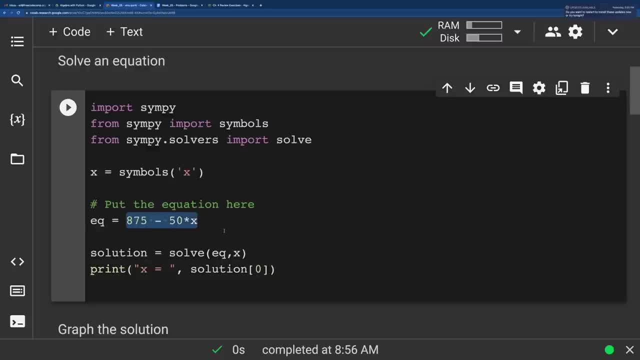 thing we needed to do here. we keep this equation variable. the only thing we need to do is put your equation there. In this case, I'll put it here: h75 minus 50x. And remember, um, it's remember the. 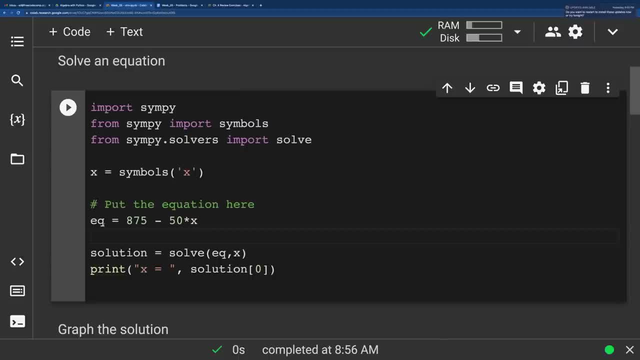 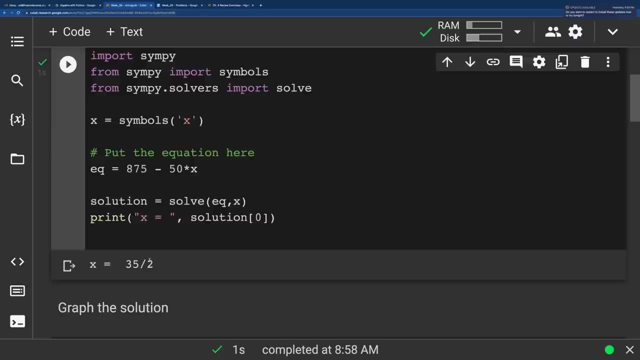 python 50 times x, So that's by default set equal to zero. so when we run it, so the answer is 35 over 2, interesting that it gave us a fraction. but there you go. so that's. 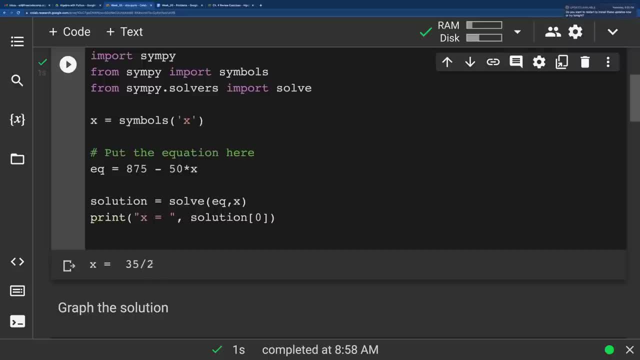 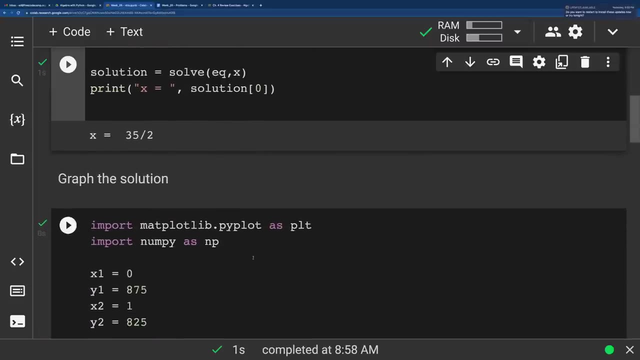 17.5.. So 17.5 years, um, it's gonna be zero. Yeah, Now again fictional numbers. I feel like you know, in 17.5 years from now, nobody, it's not gonna be that. 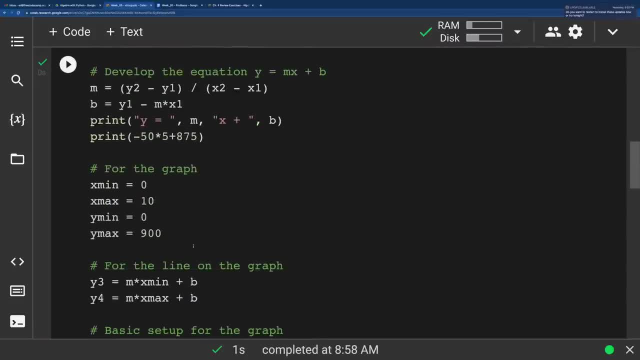 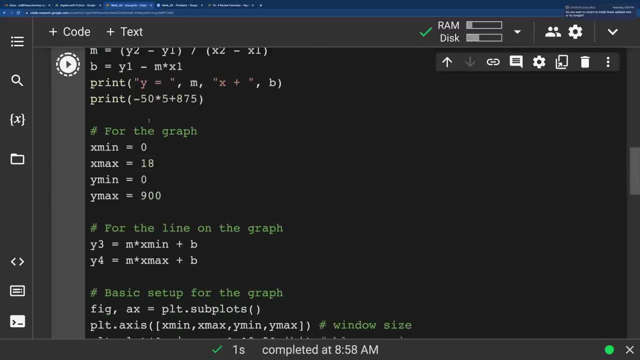 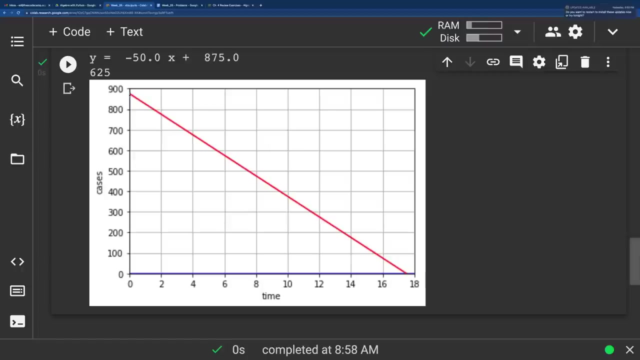 nobody has the flu or something like that. But we can actually take a look at this and we can change the x maximum to 18. And then we can see this trend. so we look at that. You see, Then, according to this trend, 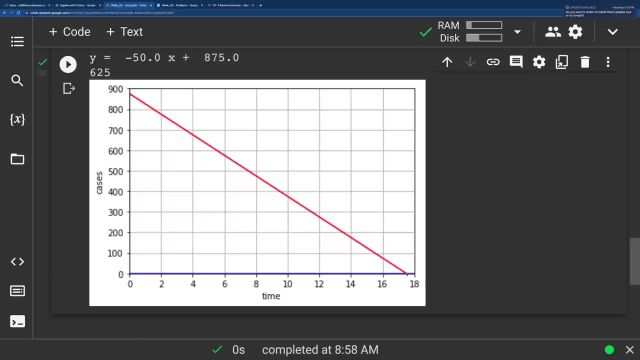 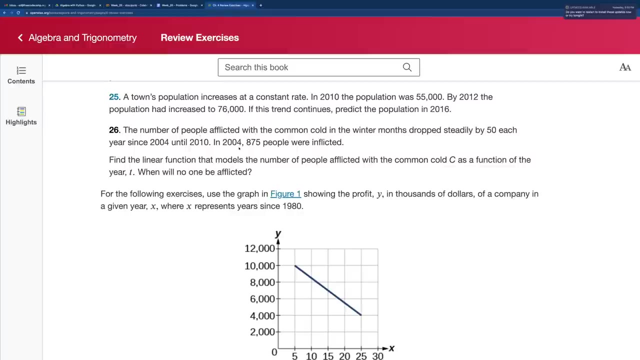 you know, times zero, and that would be, you know, 17.5 years And in this case, according to these numbers, um, who knows it may in some particular town, but in 2004,. so 17.5 or 18. 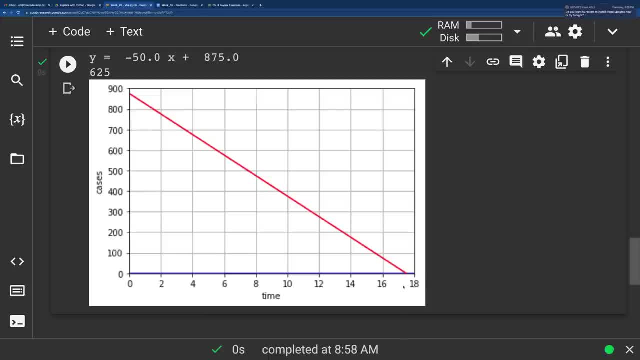 years, that would be like 2022, and, um, yeah, I feel like that would. it's not that there's nobody afflicted with the common cold, Alright, but anyway, you see the trend though. We see, you know. 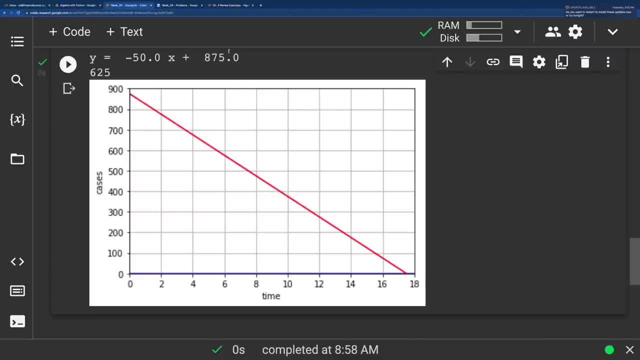 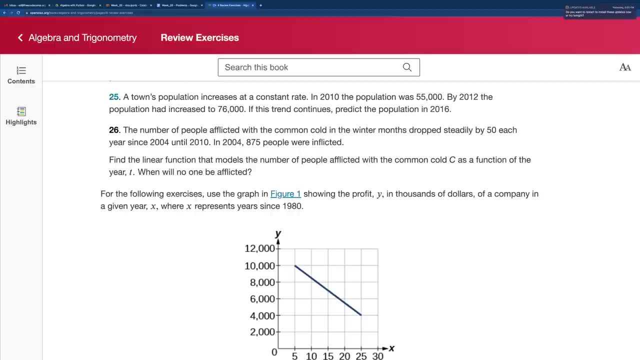 these are realistic enough that we can use these to take a look at how we would solve these, and this is what we want: to use this math for predicting trends, given the information that we have. So here's another one where they even 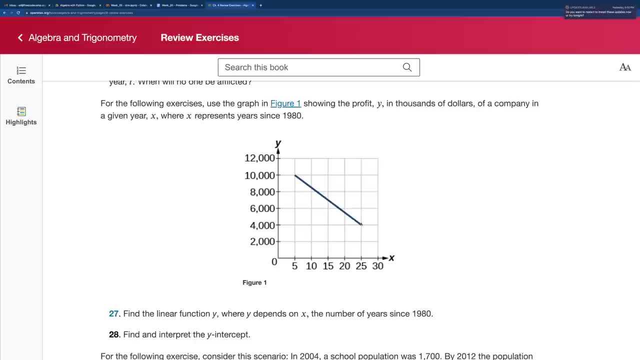 give you the partial line based on the graph they have. Alright, so this is showing profit. so this figure one is showing profit in thousands of a company in a given year. x, And they also do. x represents years since 1980.. 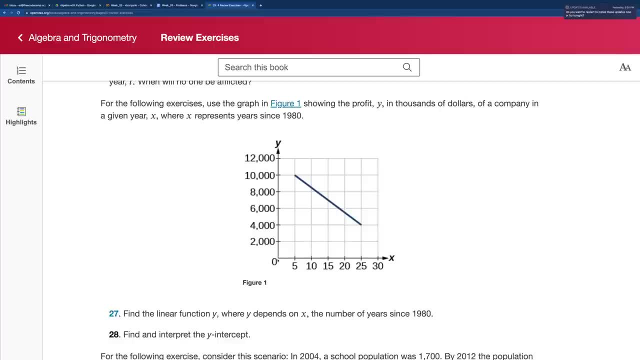 So there we go. if x, if times zero is 1980, so then 20,, so 20,, that would be 2000, and 30,, that would be 2010.. We see, you know, there we go. 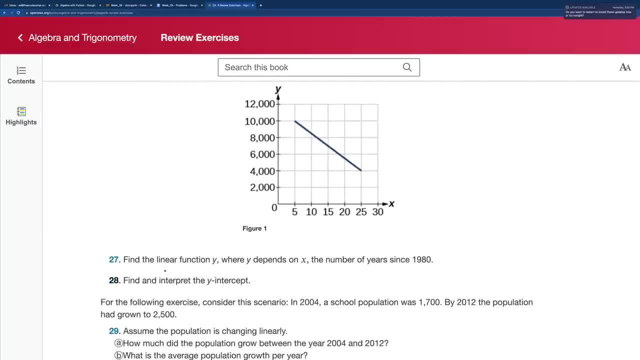 Now, given these, we want to find the linear function Alright, so let's take a look at. if I want to look at these. I just want to find two nice points that I feel confident that I'm not just estimating the points. 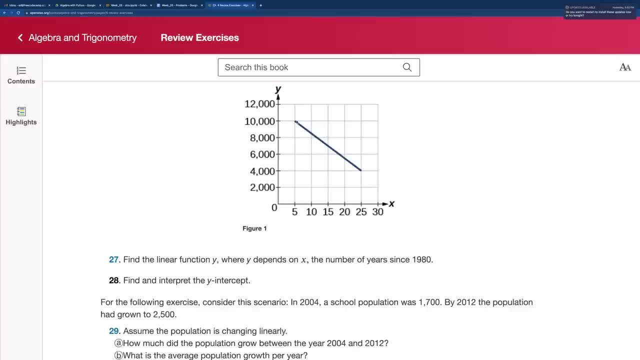 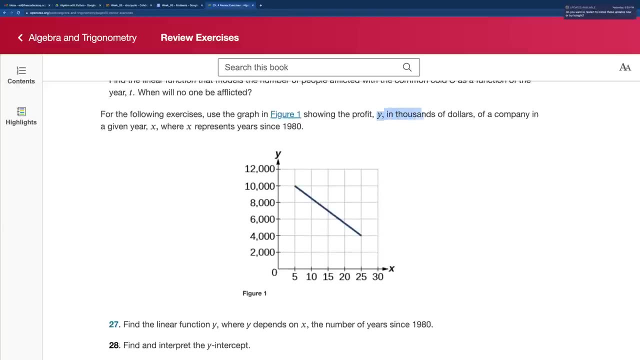 So I like this first one at at year five it was 10,000.. Now it. it's interesting because it says y in thousands. So therefore 10,000 would be 10 million. You see, So if y 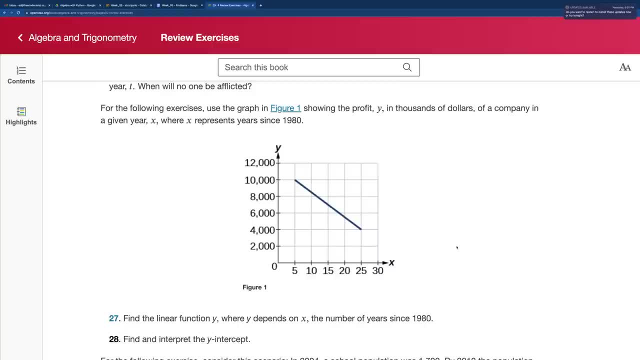 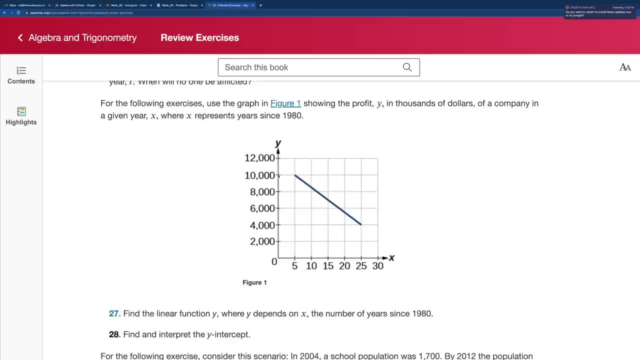 is in thousands, then 10,000 would be 10 million, In which case they could have just said it was in millions. but that's okay. Um, and then we have so five. I'm going to shift it to millions. 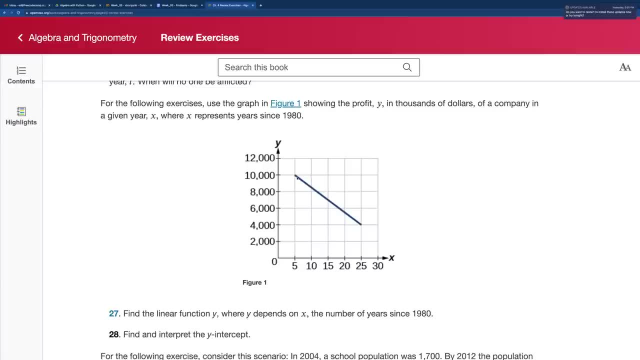 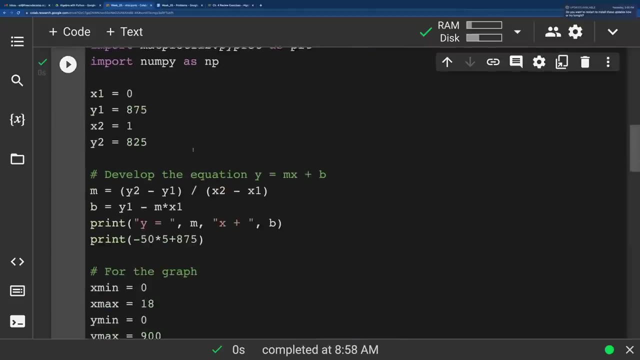 and just make the y value 10.. So 5,, 10, and then let's find another nice point. I like this: 25, 4. So we can go back and we can plug in in these, So I don't. 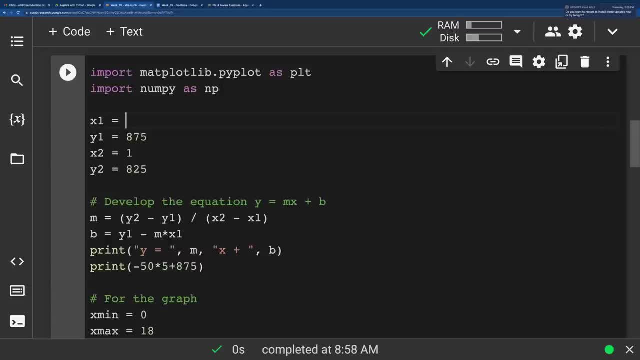 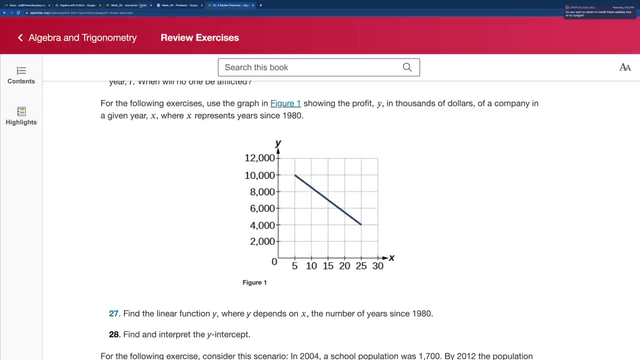 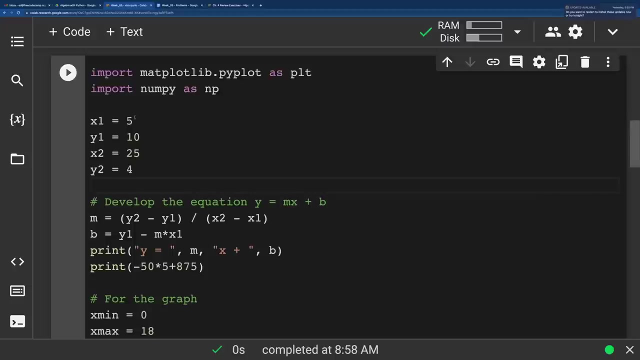 have that zero value and we're probably going to want that at some point. So 5 years, then we're talking 10 million, And then at 25 years, then we were talking 2, 4.. Okay so, 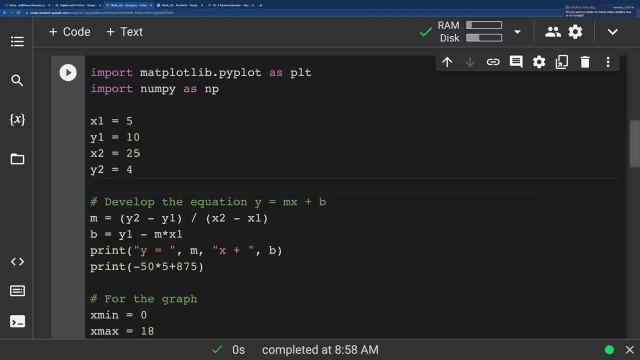 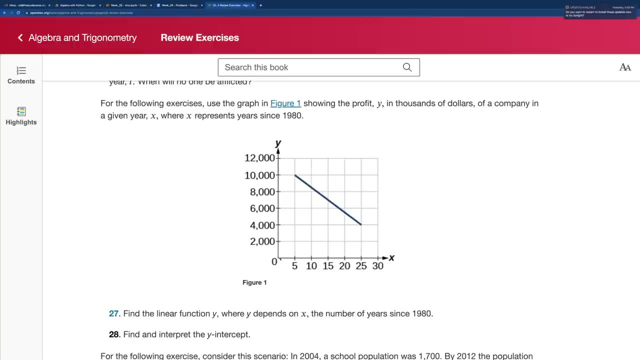 there we go. We have that point: 5 years, 10 million, 25 years, 4 million. and since we already see this graph, um, since I made them 10, I really could now we could take a look at this and say, oh yeah. 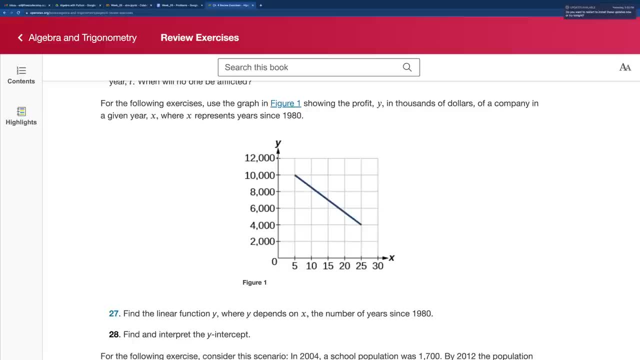 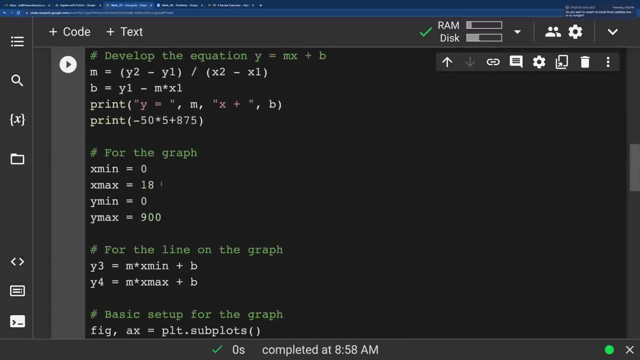 12 is probably fine as far as a y maximum, and we could continue this to 30, or, um, you know, we can take it further. So when I go to graph it, 0, x maximum, 18 is not going to be enough. 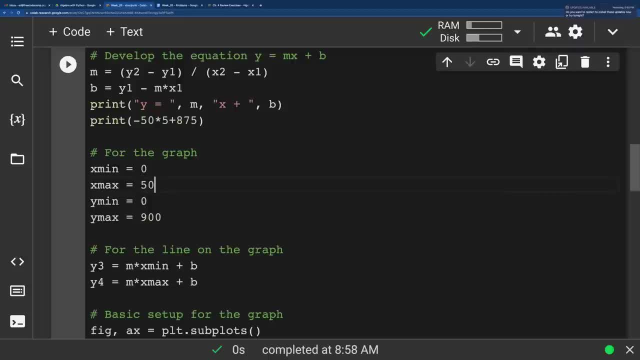 Um, maybe I'll just make it a nice round: 50, y minimum: fine, y maximum: 900.. That would the scale would be so much it would. this would just be in the tiny corner of the graph, So maybe we'll just call that 15,. 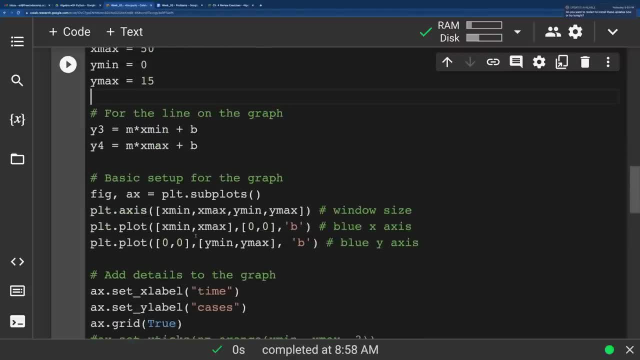 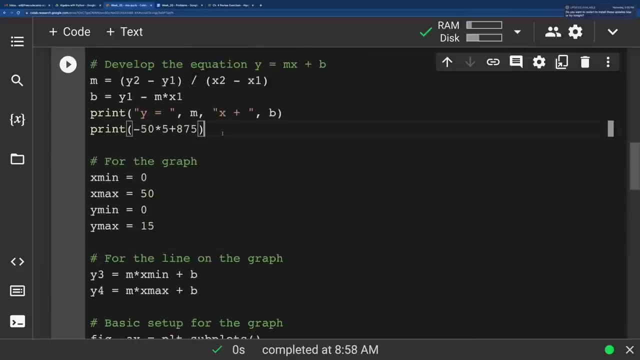 or something like that. Alright, there we go, And for this one, we could, we could, we could just delete this, just delete this. like the space in there, like the space in there, we could just delete this. and we have. I'm going to print out the. 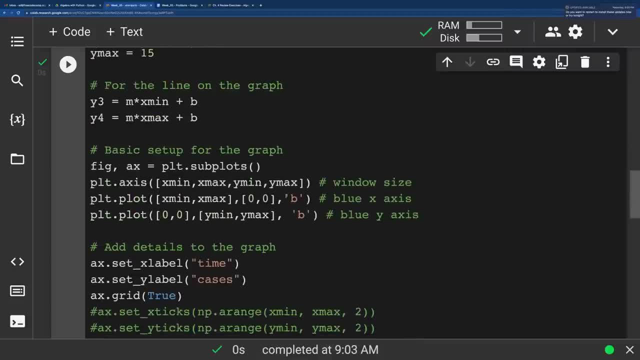 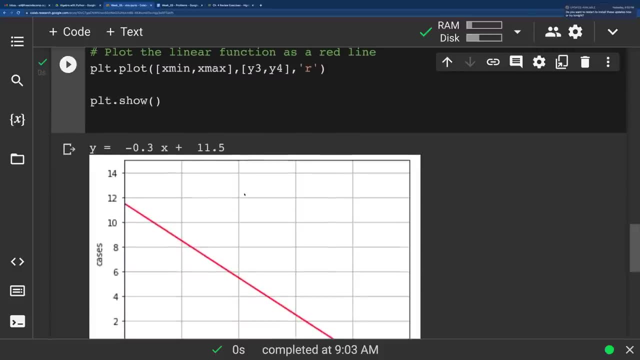 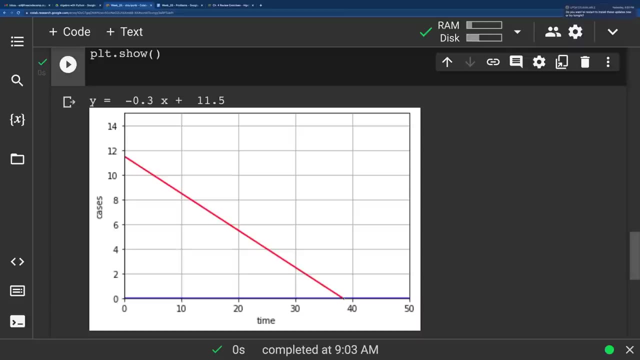 the equation, So when we run it. so here's our equation: negative: .3x plus 11.5, .3x plus 11.5, and we see this downward trend over time. And here's another one where, if I wanted to, 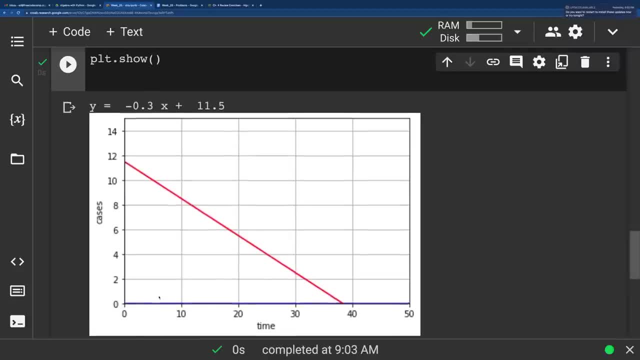 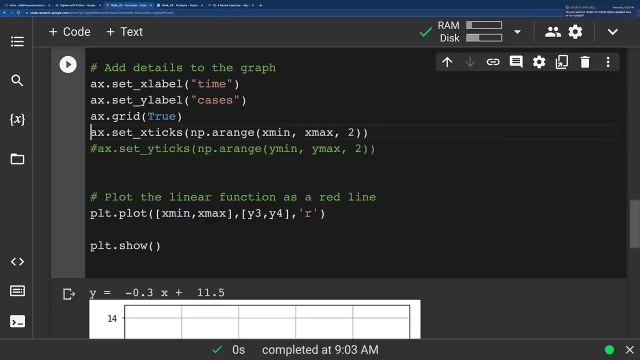 change these tick marks. maybe I could change this to the x ticks: is two enough? Yeah, Yeah, maybe. and then I can change the Y ticks: Is 2 enough? Yeah, maybe. We'll see And we'll run it. 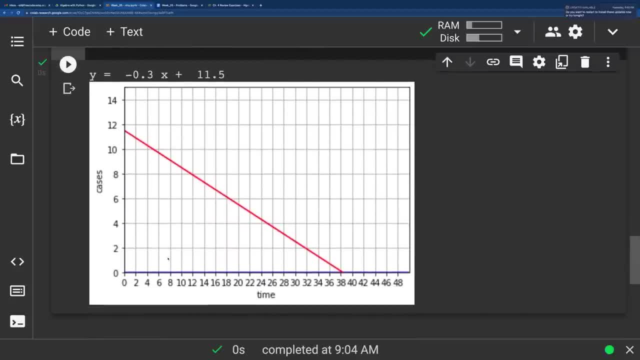 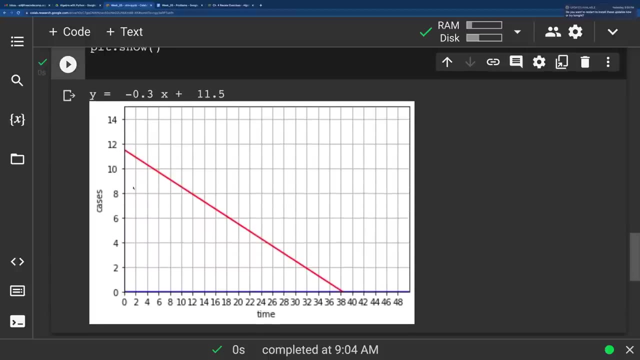 So we see we get many more lines, All right, And with that we see that this is 38. Now, just because these end up being rectangles more, I might change my Y ticks to 1.. I think I just like that better. 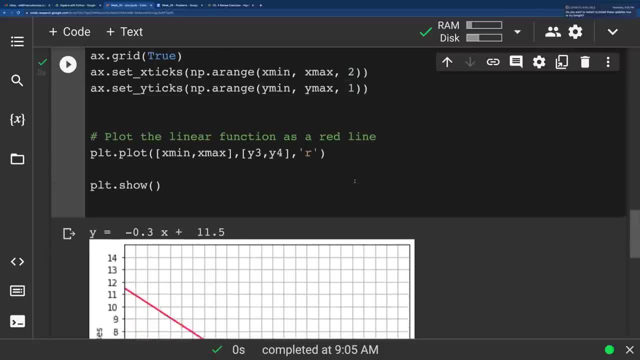 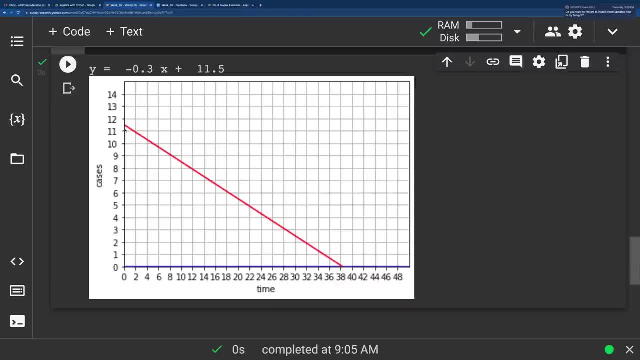 And you know, in doing this you can, you know, change some things and go There, we go. So with this, then we can really see the trend. There's your 11.5.. And then we can see this downward trend, down 0.3.. 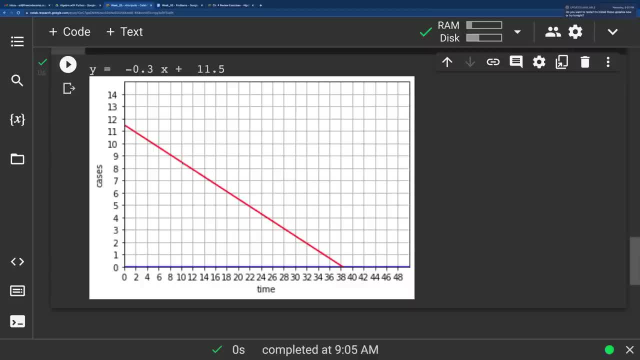 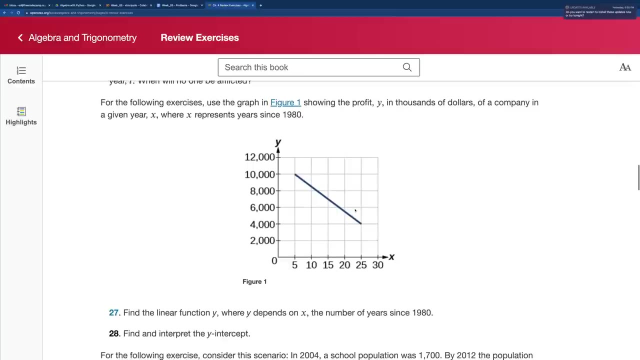 So it should go, you know, over 10.. It just went down 3 to 8.5.. And then, 38 years later, then they would have no profit, because that's the trend that we're saying. There we go. 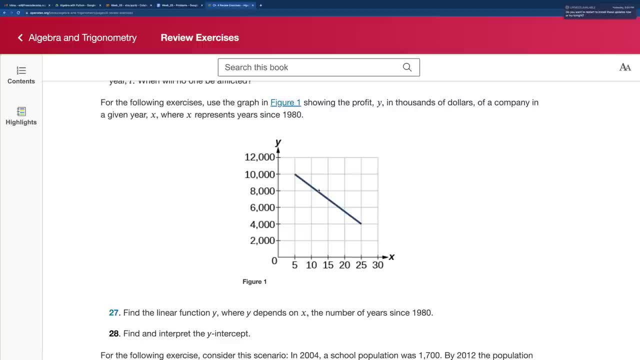 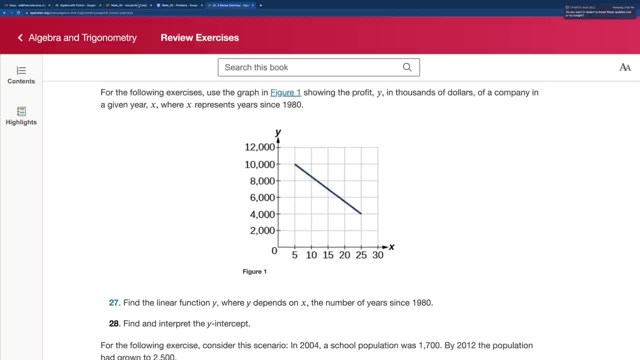 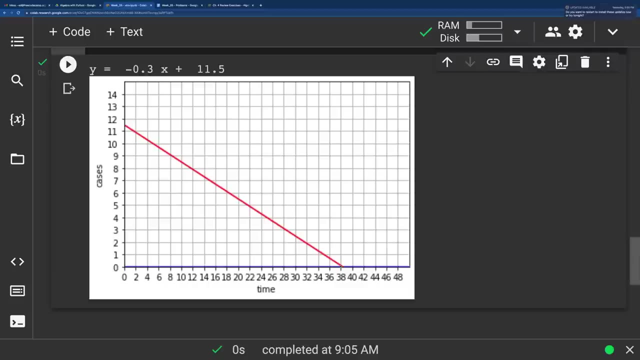 So, whatever this company is, this is their profit since 1980. And then there we go, 38 years later. then they would have no more profit. So who knows, Who knows what company this is, But you know our fictional company is. you know, something would have to change. 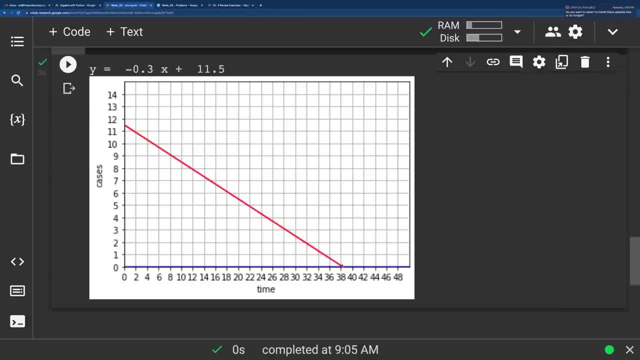 But that's where the prediction lines, you know, the simplest prediction is: okay, these would go in a straight line. Whatever trend would continue in a straight line unless something changed. But we know then, in normal business, normal day-to-day life, things do change. 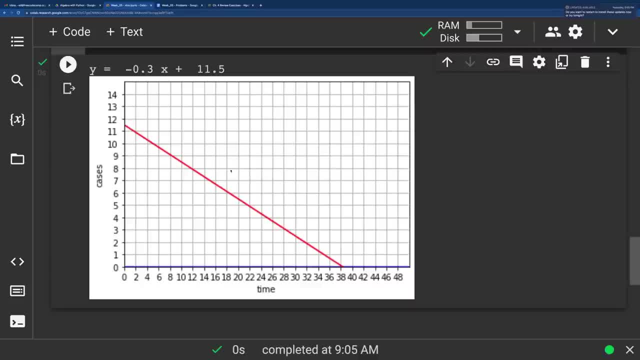 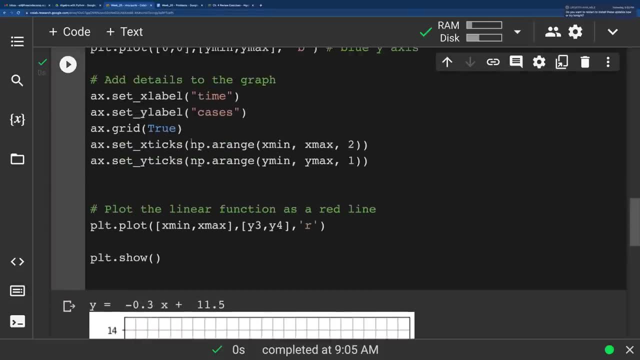 And that's why our lines aren't always perfectly straight. But This gives us often enough of a prediction. Oh, and you see, then time and then cases, Then we would change that to profit. Okay, Just to make it official here. 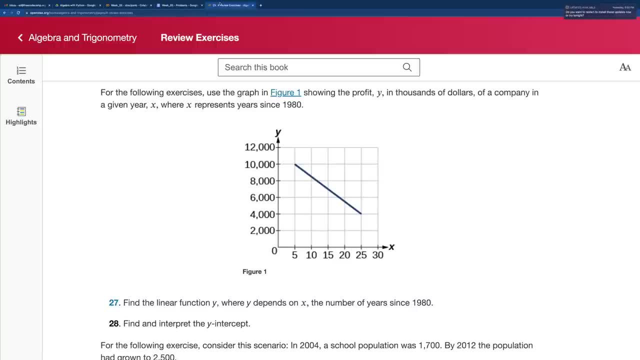 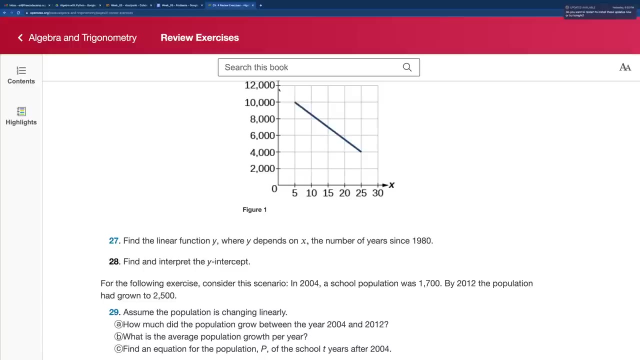 Time and profit. So there we go. So another situation And we can see where it would start, And then Profit declining. And that's enough years that you know. 11.5 million was a lot more money in 1980.. 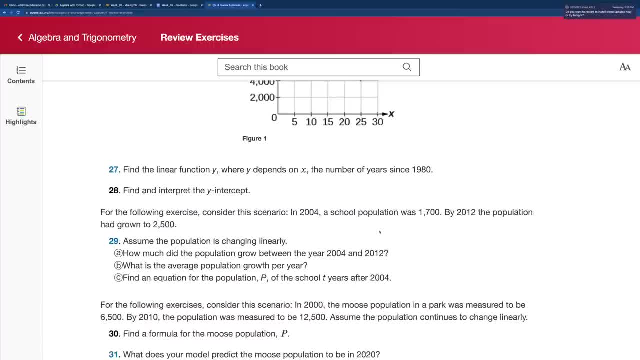 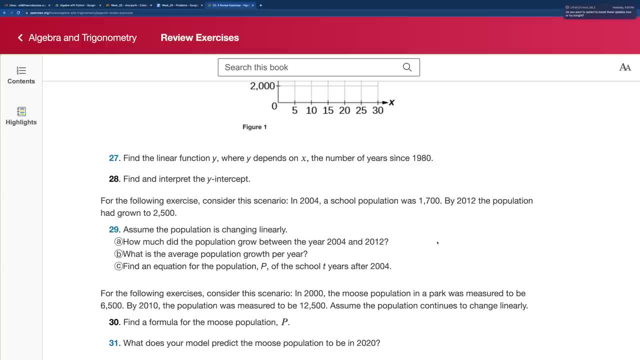 And then profit declining And Yeah. So this company is definitely whatever they were doing there. You know, they were in sad shape, All right, And we have the Y intercept and all that. Okay, So we see another very, very similar. 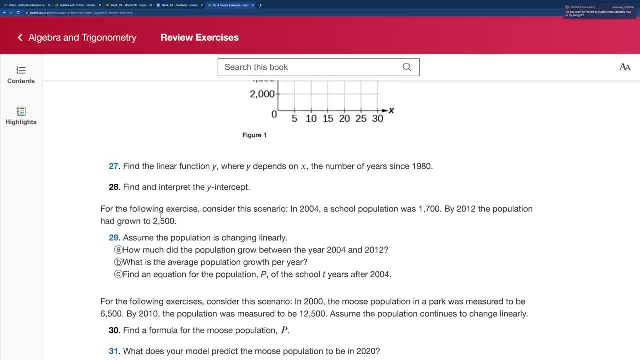 We'll do one more here. So consider this scenario: 2004 school population was 1700 by 2012.. The population had grown to 2500.. So all right, And again assume. assume the population is growing linearly. 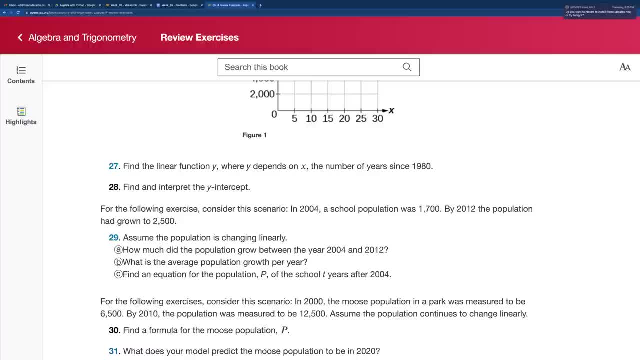 All right. Now how much did the population grow? So this a is really just the subtraction. So 2500 minus 1700 is 800.. So it grew that much. And then the average per year. you see Anything per year, the rate. that's the slope. 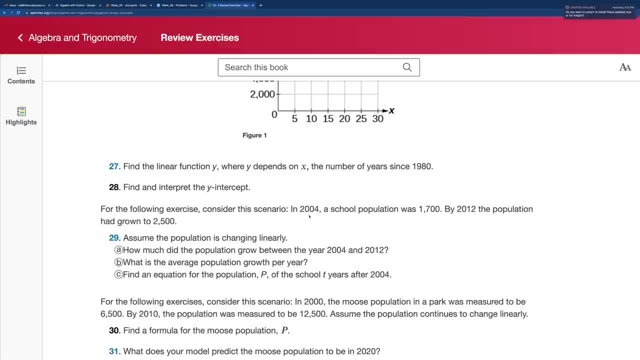 And we can divide that, but we're also going to then just plug these numbers in and you'll see that we can see the slope. So 2004,- maybe we'll call that time zero- 2004,, 1700,, 2012,, 2500.. 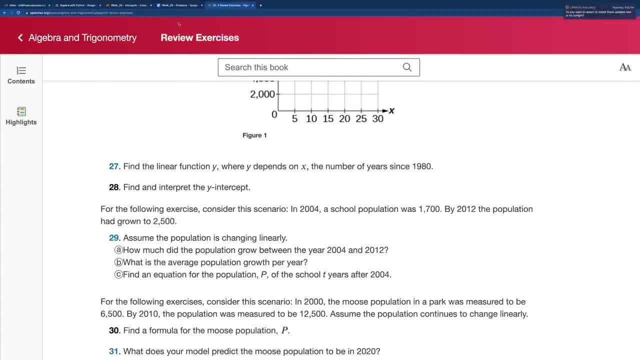 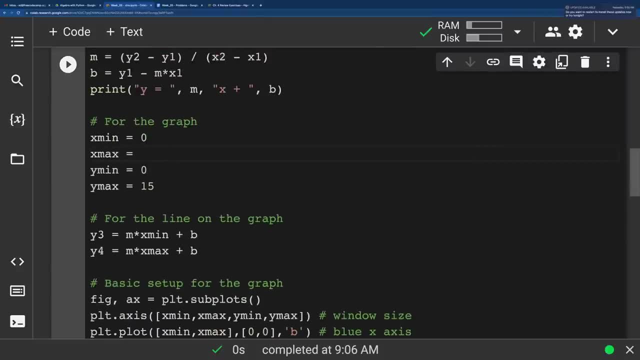 And I might even leave the hundreds because we want it to be, you know, more exact. We know that the population would be continuous, It wouldn't just jump hundreds. So 1700.. And then Y minimum, And then we have 2500. 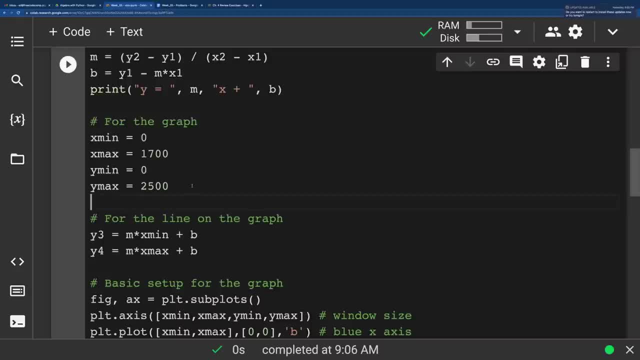 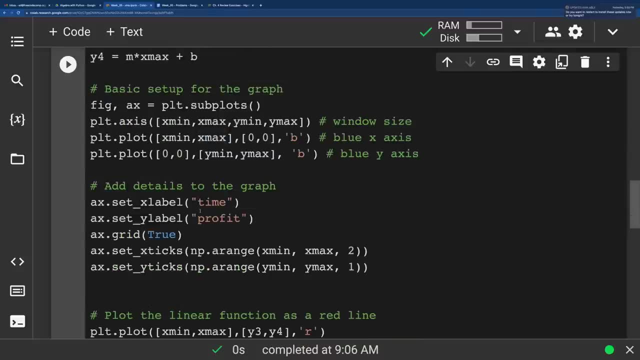 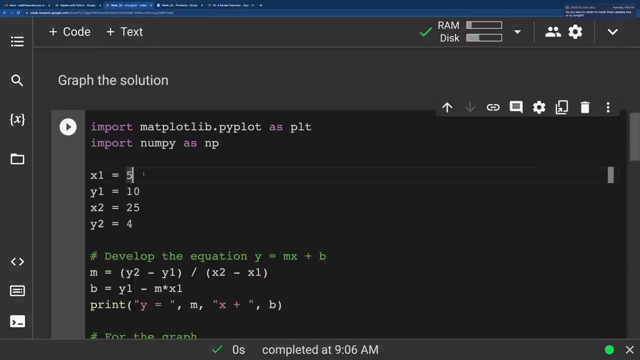 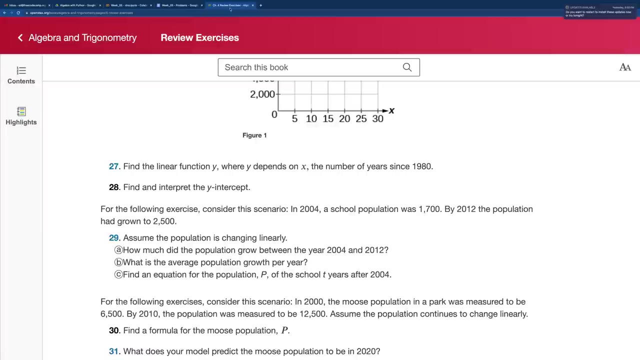 So then, after this, if I wanted to F this, Then My Y maximum On the Oh I put in the wrong. So there you go. Time zero: 1700.. And So in 2012.. 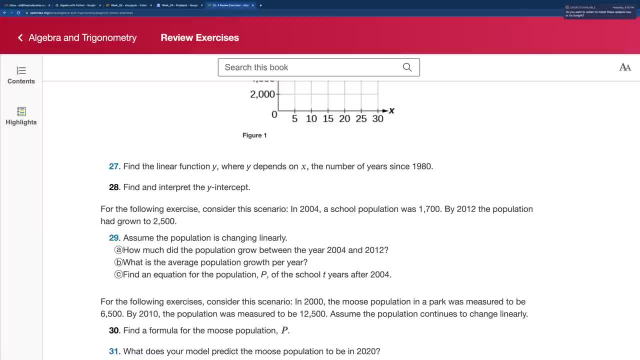 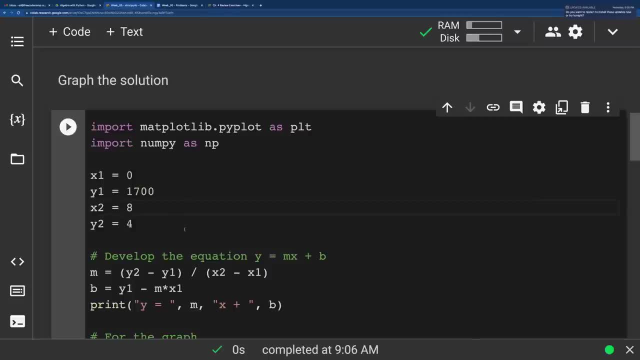 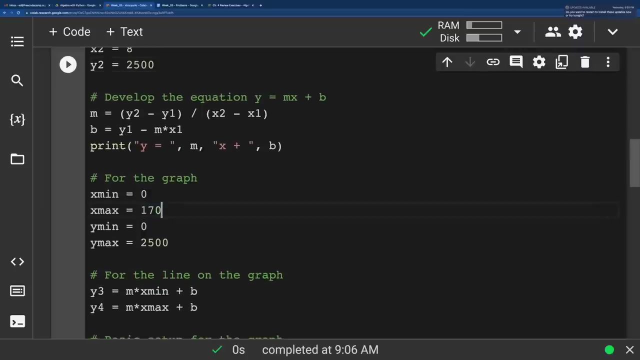 So Time zero, And then in 2012,, so that's eight years later, it was 2500.. So eight years later then it was 2500.. Here we go. Okay, so we'll have that and X minimum and then the X maximum. 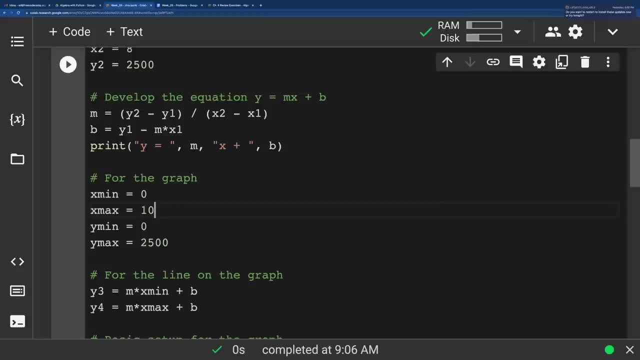 So let's just make it a nice even 10.. And we could always change it if we need to. Why maximum 2500, but we're going a little bit further. So let's make it 3000 and see if that's going to be enough. 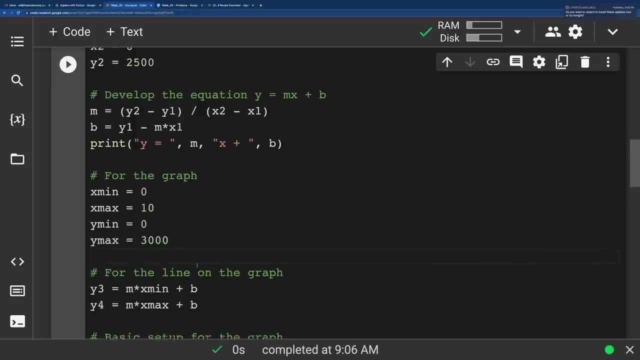 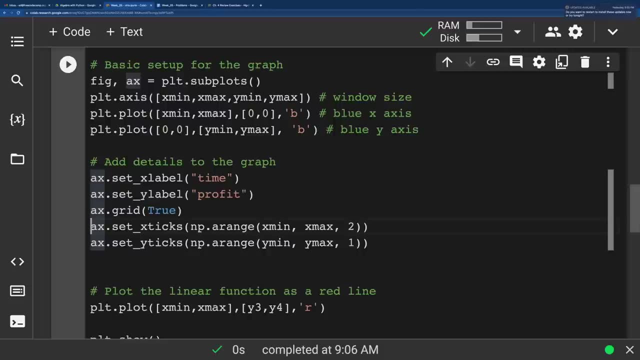 Oh, Here we go And Do. I want the ticks for right now. See, if you comment them out, the graph will. The graph will, as we saw, it will still give you The, It will still give you the tick marks. 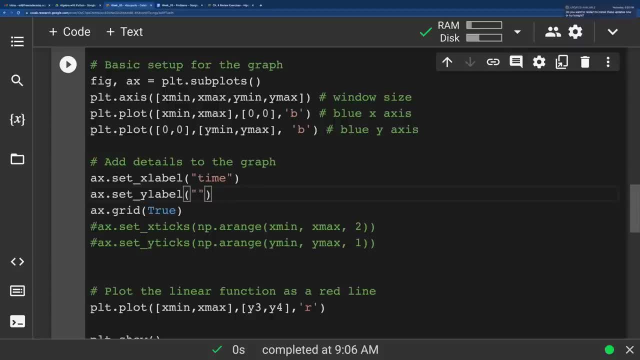 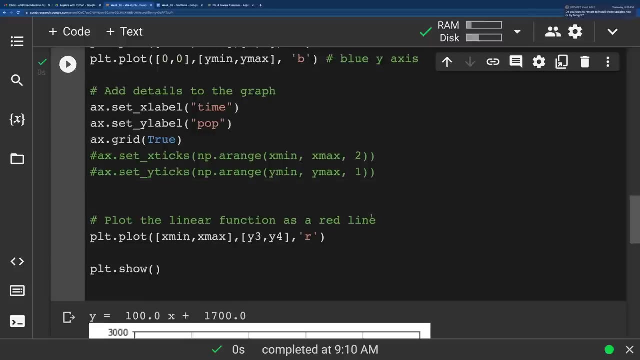 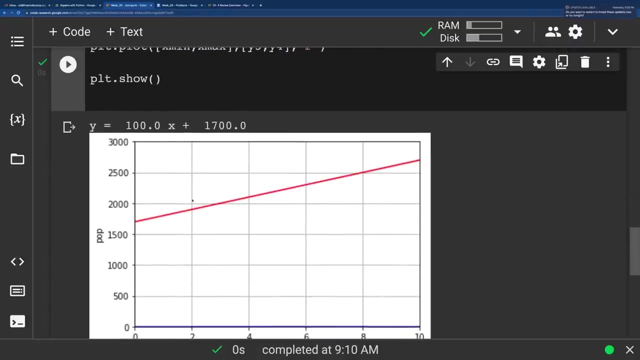 It's just that the default, whatever Python wanted to calculate and where you can force them into However often you want, There you go. And For school population, Yeah, All right. So we see it's growing by about a hundred a year. 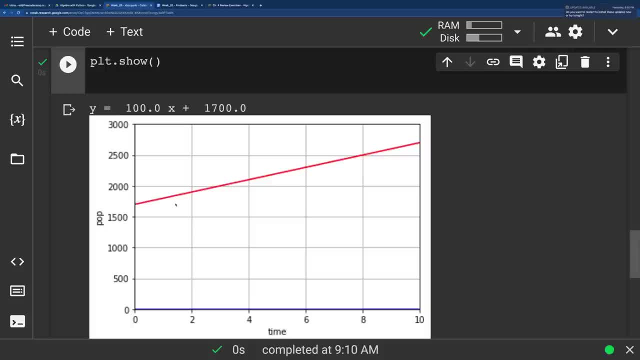 And maybe that's you know, depending on what you wanted to estimate, These tick marks might be fine, The grid might be fine And You know, if you wanted to, you could always Add one More. change it, You know, I I think that works out. 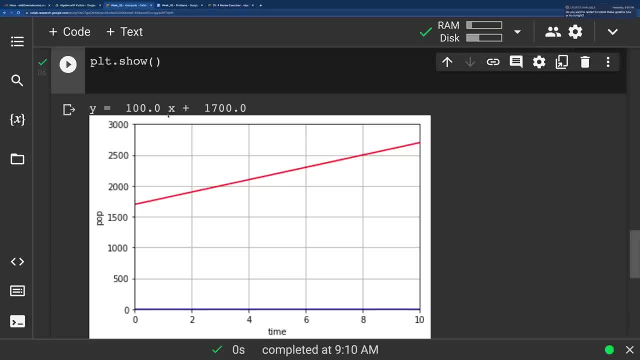 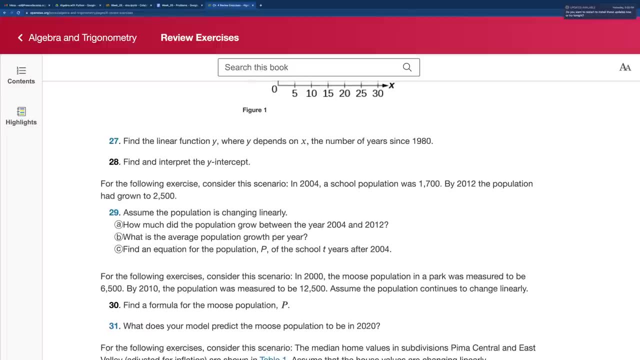 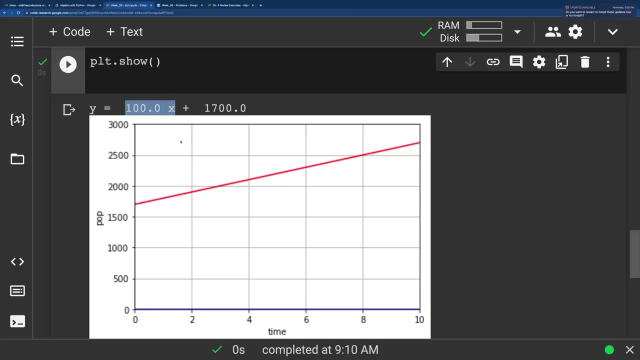 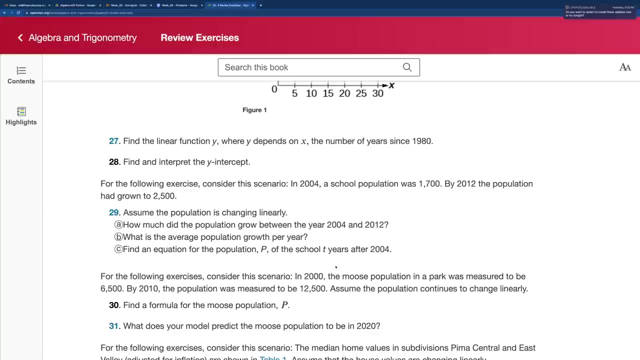 So Growing by a hundred every year And we can use that to predict. So the average populate growth per year was a hundred. There we go 100 X, So the slope is a hundred And there's the equation for the population for two years after 2004.. 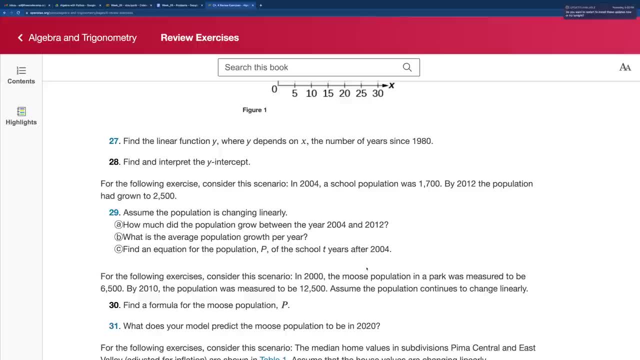 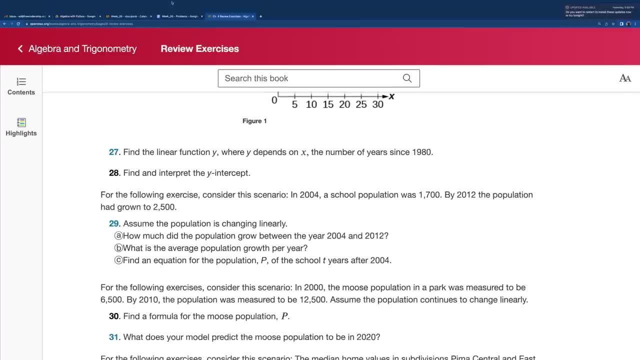 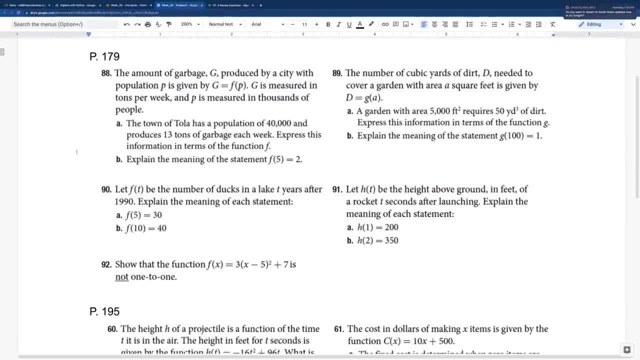 So we see, you know, we, we've done a few of these. I think I, I think we don't need to do another population model. but there's some other form, There's some other practice problems that we see in other tech. all these, all these are coming from that textbook, the second textbook, algebra and trigonometry, because there's a lot of good business applications in it. 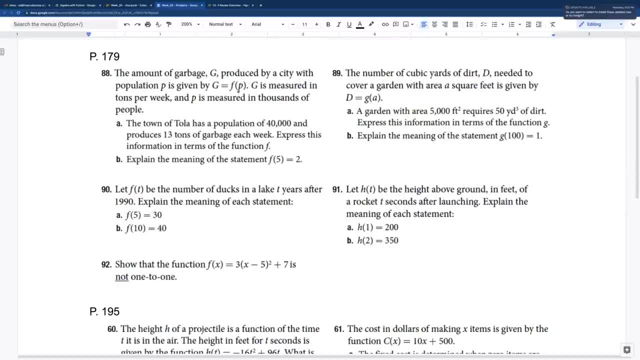 So you know, here's, Here's the idea that just the notation um G equals F of P, the amount of garbage G produced by a city with a population P. so we can go: a G equals F of P, and that's how we would read that. 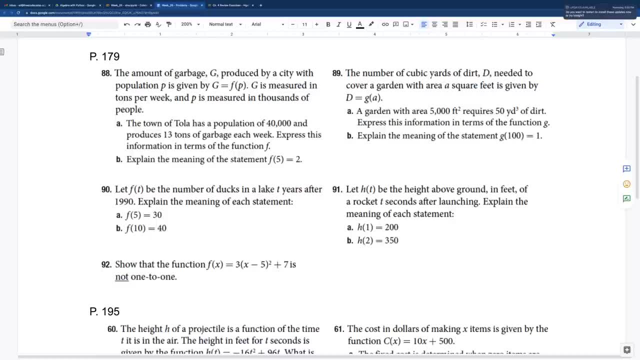 So it's a function of population And what that tells us is population is the independent variable And then garbage is the dependent, and Population very often is an independent Variable. that causes a lot of other trends. so we look at that and we see the same type of thing. the town of Tola has a population of 40,000 and produced 13 tons of garbage each week. expresses information as a function. 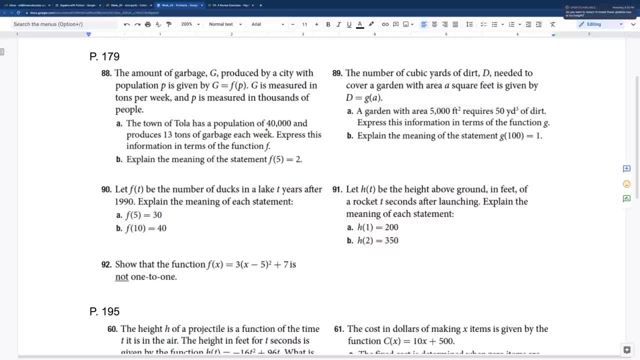 So Now, If we have this Um, One of the things that we Would guess is that If it's a function of population, Then No people would mean no garbage. So in our Y equals MX plus B, scenario B would be zero. 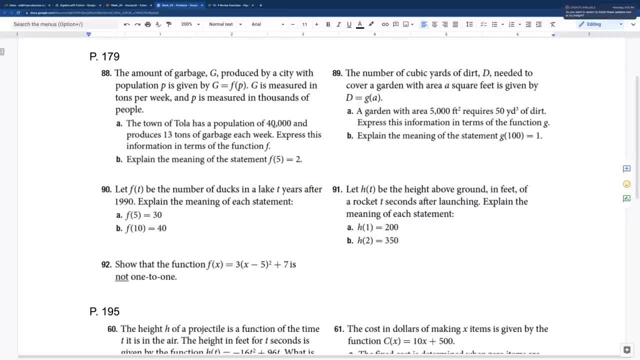 And notice we, because we only get exactly one point here: 40,000.. 13 tons. So If we, If we wanted to set this up, you know, we want to look, you know we know that we have the 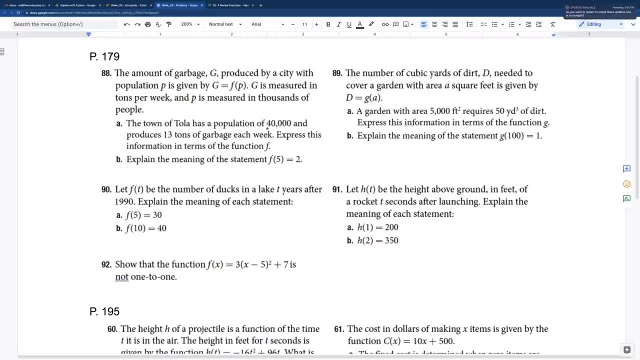 Python scripts to solve this. but if we want to set this up, We want to take a look at How we're going to set this up. 40,000 is going to be the population and, who knows, maybe I might just call it in thousands. 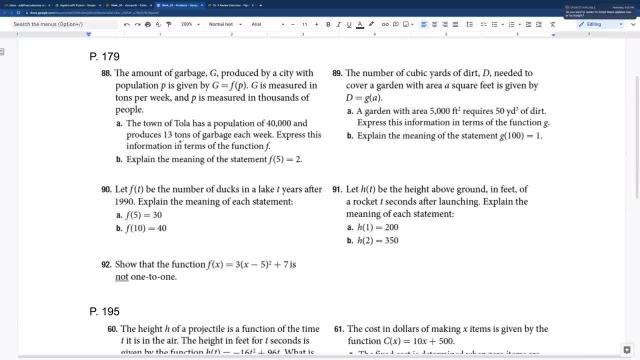 And then 13 tons Same thing, I'll just call it 13.. Um, And Then we say, well, that's one point. Where do I get the second One? but we have to look at the situation. Would I think that it would start at zero, zero? 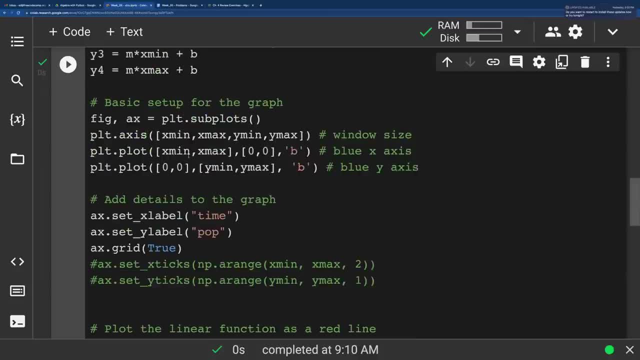 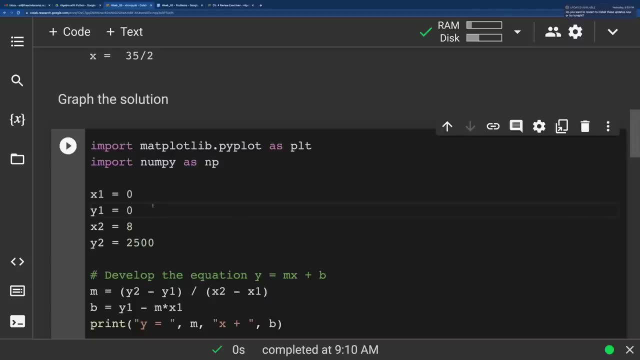 And if that's the case, then we could go back and say so: here's zero, zero. And then, remember, our X values are going to be population, So we'll call that 40. And then that's going to be 13.. 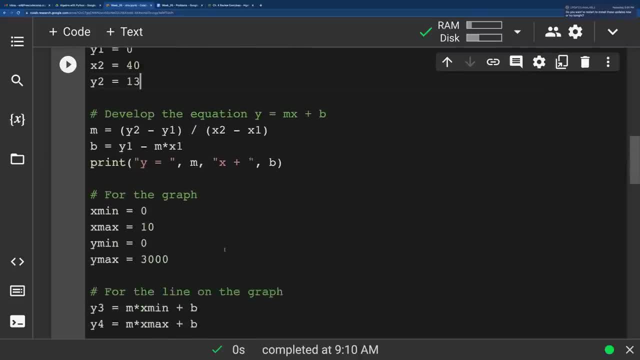 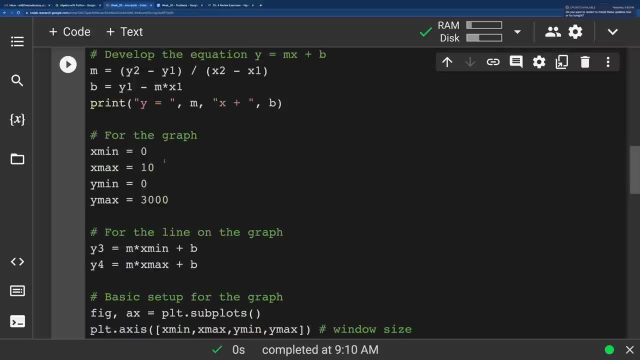 Because It's in tons, And therefore the X minimum zero, fine, but X maximum um 40 is probably not even enough, Cause we start with that and we can expect that it increases. So then Let's say the X maximum. 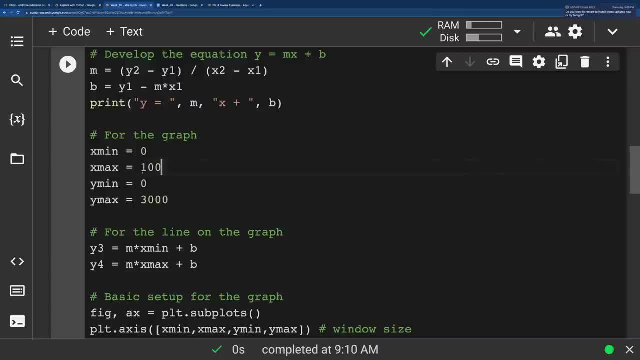 Would be, I don't know. let's make it a hundred and we'll see Why. minimum zero now 13.. Um, maybe make it like 50. We'll see, See if that's enough. of a Y maximum. So there we go. 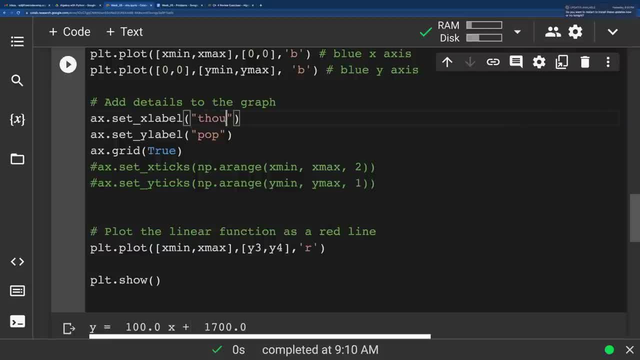 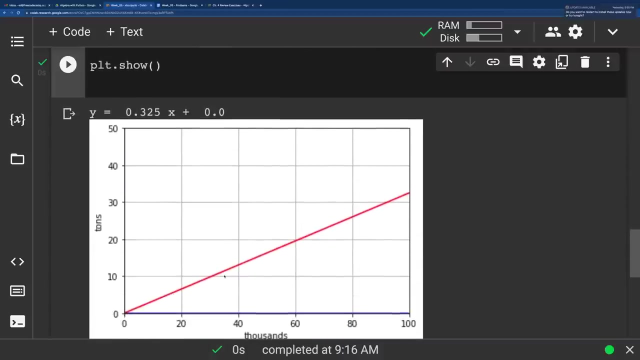 And We can just write this in thousands, And we can make this in tons. So thousands of people, tons of garbage. So we have this trend here. There we go: 40,000 generates 13 tons of garbage, And we can see this trend here. 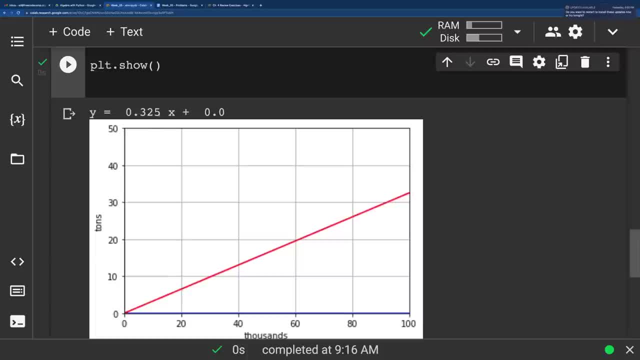 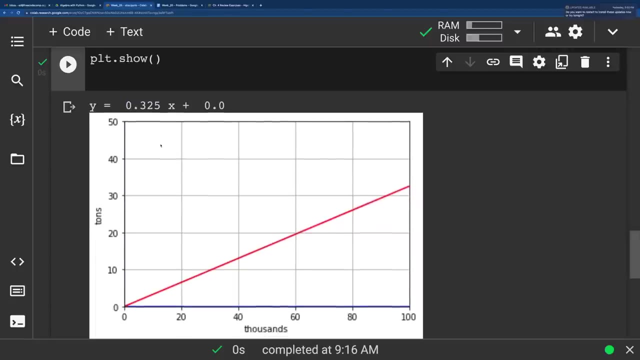 Okay, So there's the rate here: 0.325 X. So remember the X value is in thousands. So every thousand people, according to this fictional scenario, makes 300.325 tons. So So that would be about tons, 2000 pounds. 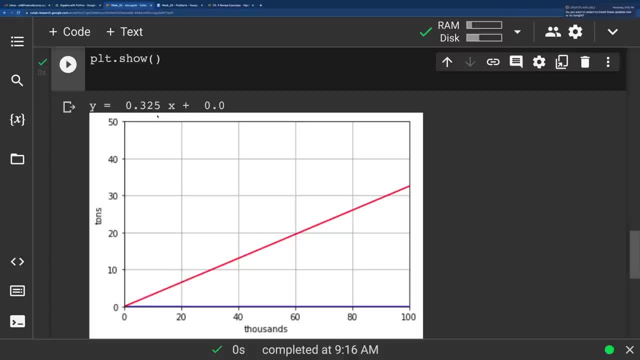 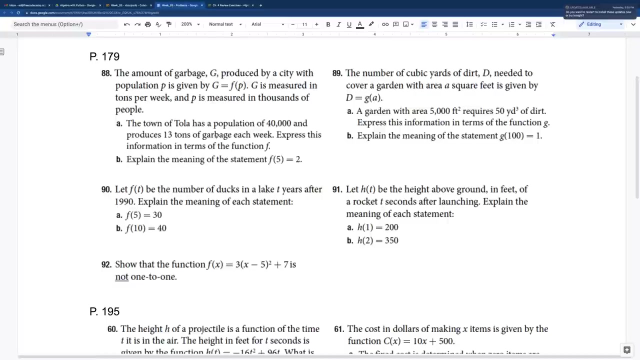 So that times 2000 would be about 650, but then if that's thousands of people, so that's each person making less than a ton of, less than a pound of garbage, Maybe, Maybe, So. So again, this is, this is not the you know um latest research. 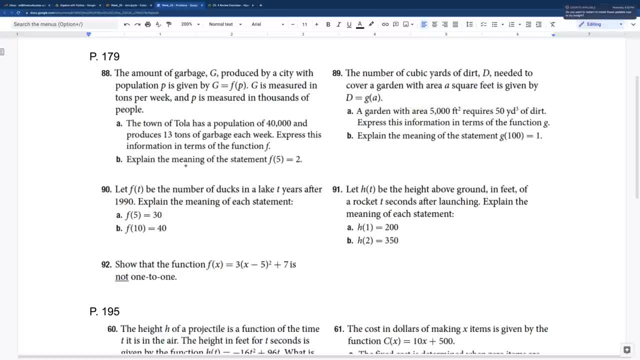 This is, you know, a couple of numbers that seem realistic. And then what's the meaning of this? And we would read this as F of five equals two, So notice that the function, like our functions in Python, that five is the input and any input, or 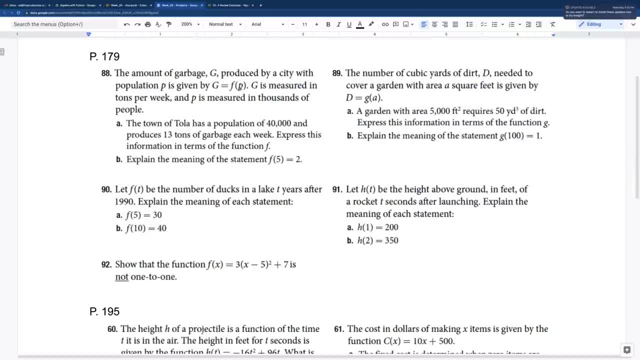 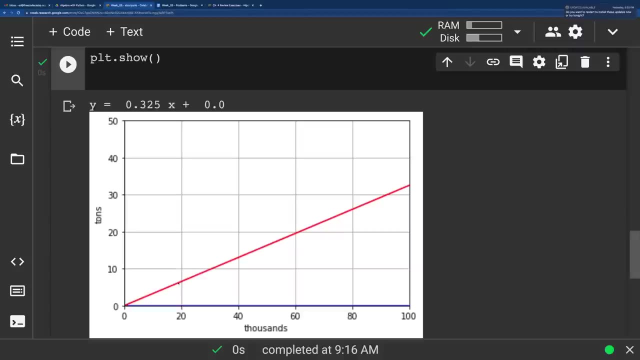 So the input is an independent variable, That's X Or you know um, even though we call them P and G here, so that input five and then output two, So F of five is two. So we would expect then that that means that when we're talking about 5,000 people, then 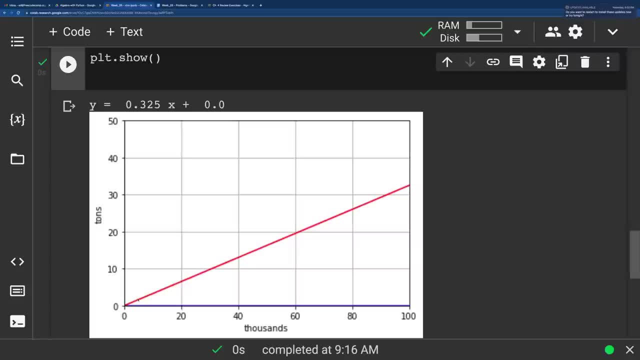 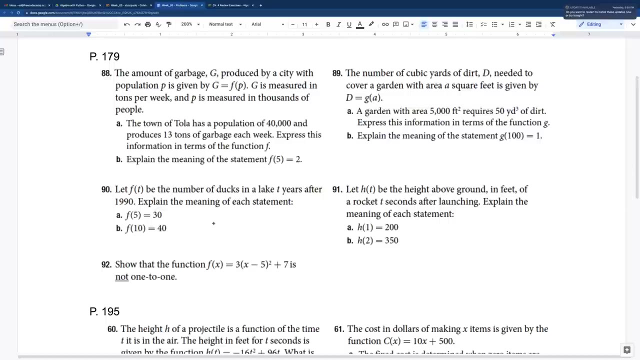 the 5,000 people would produce two tons of garbage, Right of garbage. so that's the meaning of that. you know, five is the input, two is the output. so in our x- y scenario here, that that's what that would mean: 5 000 people would produce two tons of garbage. 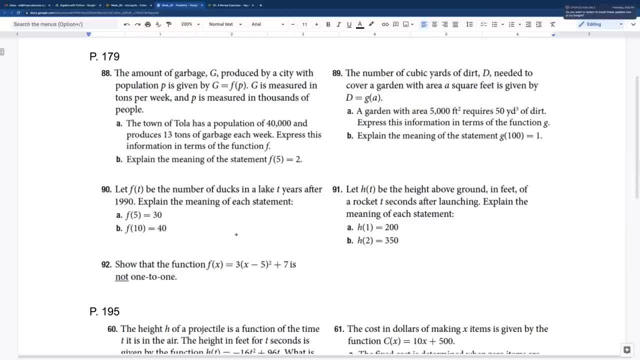 all right, and so let's go over here to 89 and another one. you see, don't get caught up in the alphabet soup of of this, as people use different notation. notice the trend of: i would read this as g of a, so it's a function of this input. a, so the number of cubic yards of dirt. 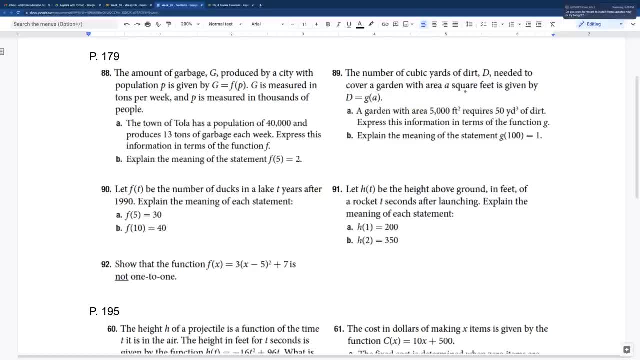 d is needed to need to cover a garden with a square feet. so d for dirt is g of a and we read like that: g of a and the common notation you'll see in just general math is f for function, and then often we just go through the alphabet: f, g, h for 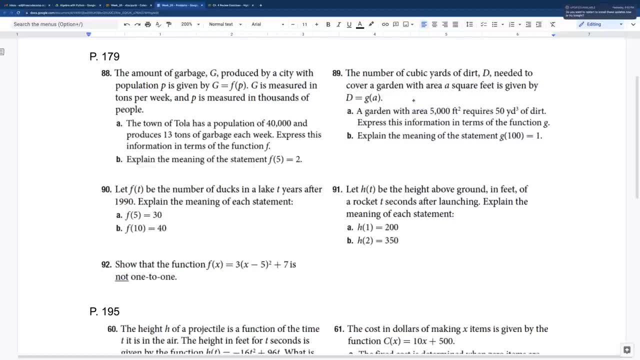 other functions we want to talk about. in python and pretty much across computer science, your function can and should have a much better name. so you know that's something that computer science has an advantage of, but nonetheless you'll see this all the time. you know g of a, so again, we 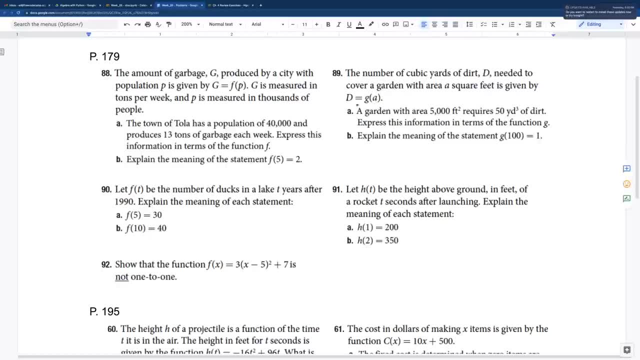 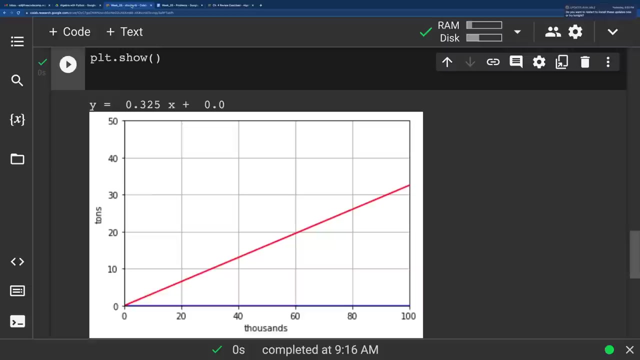 notice the trend: a is the input, that's the area and then you. given that area, then how much dirt would it be? so we have 5 000 square feet area requires 50 cubic yards of dirt, so that 5 000 requires 50. now we're not even going to do any. 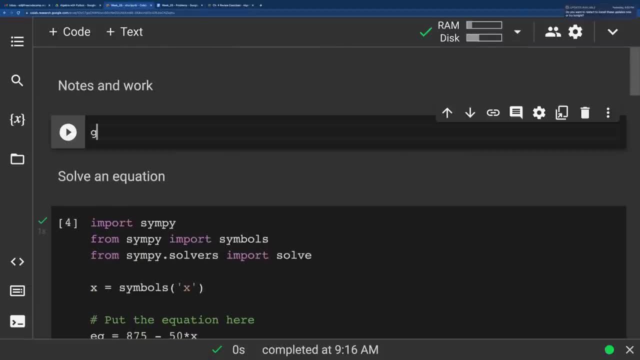 calculations to this, but i just want to show you that it that would be g of g of 5 000 square feet area, so that would be 50 cubic yards of dirt, so that 5 000 requires 50. now we're not 있지 starting with that g of 5 000. 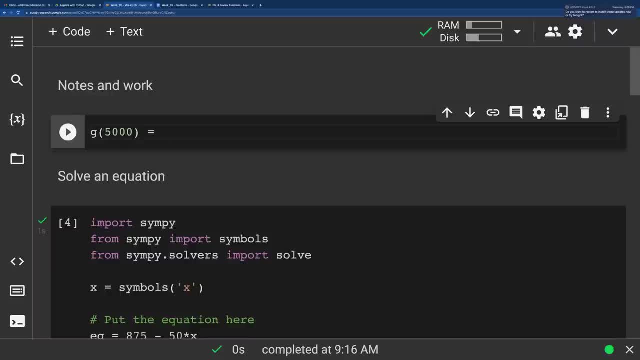 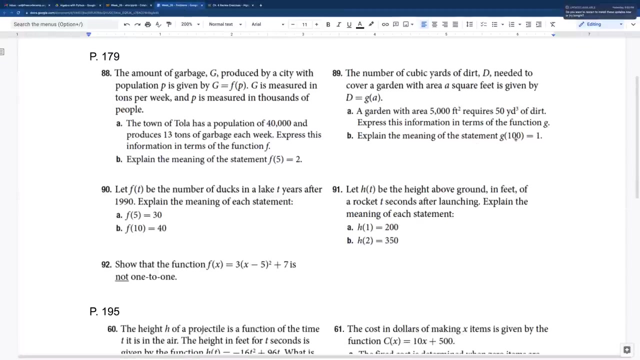 so that's just how we would write that, given that input, you'd write that the will vi, that we would know first then, therefore, how much dirt we need, and that that would just be how we would write that there's- we don't need to do any math to that right now- and the same thing: g of 100 equals one. 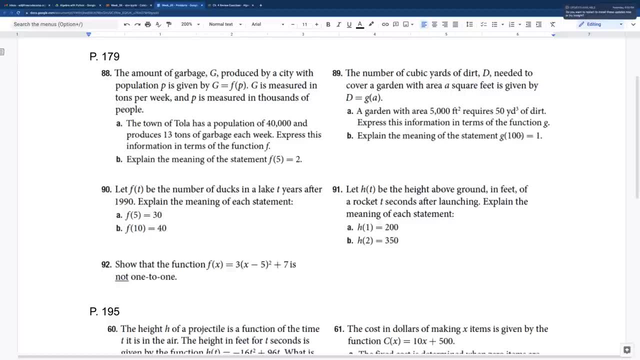 so 100 equals one and one hundred. that's the digiti ей tr Clinton now. so every how many people have ever looked up 50, something like that? you don't. cubic yards or 100 square feet of garden requires one cubic yard of dirt. 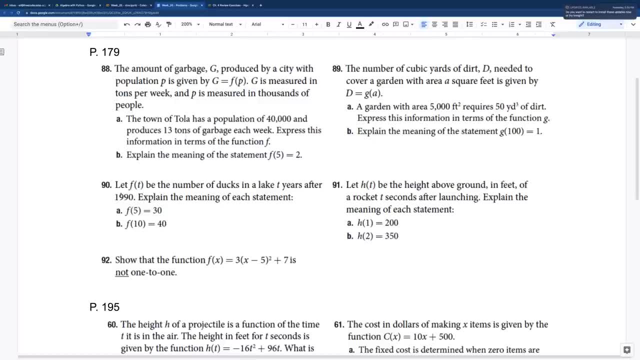 Alright, and question 90, we'll see just another situation. f of t. so there you go. some function. The number of ducks in the lake after t years, after 1990, so f of 5 is 30,. so we know 5 is the time. 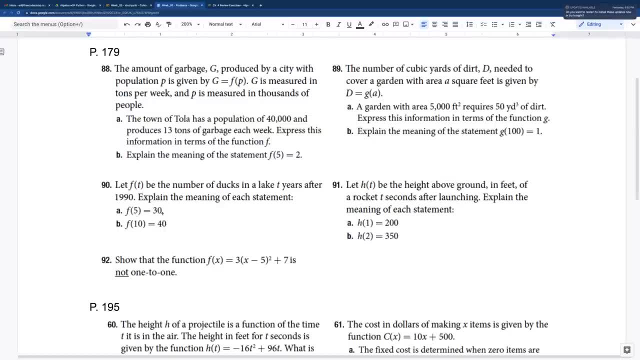 years after 1990, so in 1995, there were 30 ducks in the lake and then f of 10, so in 2000, there were 40 ducks in the lake. And given these, you see, we can. 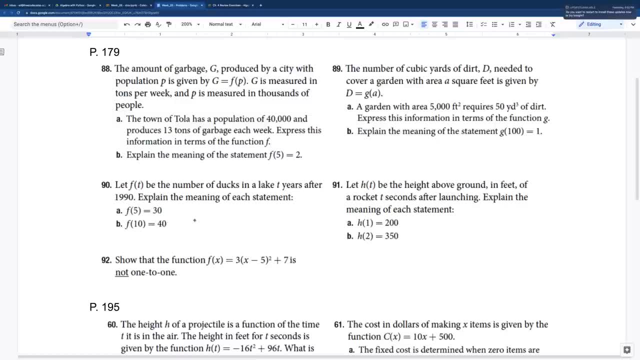 x, y, x, y. we can find the overall equation plot, the points graph. it make some other predictions, but that's the notation here and this is what that means. Alright, now 91,. the interesting thing is for: 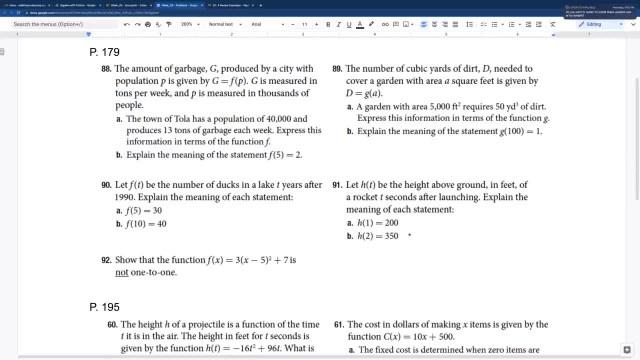 just answering these questions. this won't matter. but this is not going to be linear, But we can still answer these questions because each of these is still going to be the same. Now notice h of t and now, in this case, h for height. 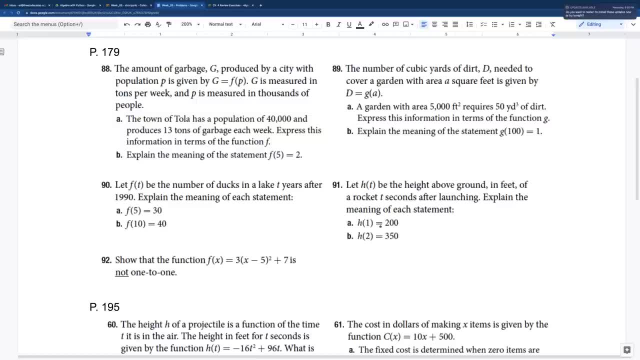 but again another way of expressing this. so as x, y values, x is 1, y would be 200.. The h of 1 is 200, so that x value is t for time in seconds. so after 1 second it's 200 feet up. 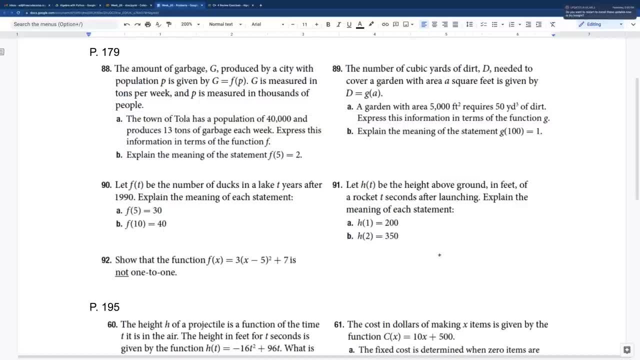 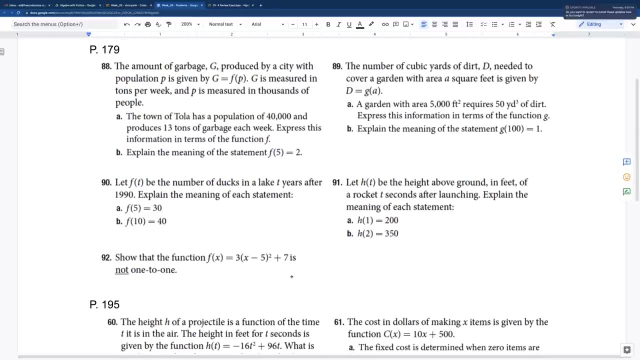 After 2 seconds it's 350 feet up, And again this is not linear, so the same things that we've been doing actually won't work for this, but we can still get the meaning of each statement here. And 92, the 1 to 1. 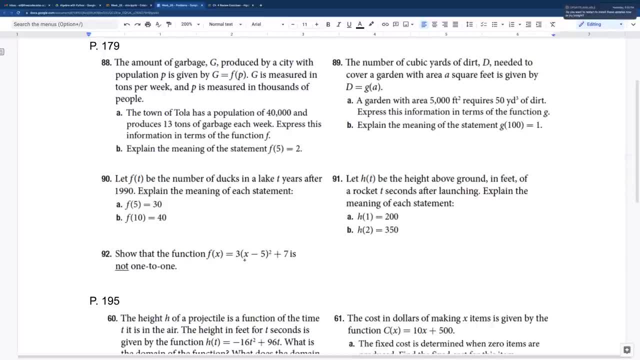 is- this is still a function, but that each x value and y value pair up like neither of them show up again. But this is a parabola, because we see x squared and we'll talk about parabolas later. But 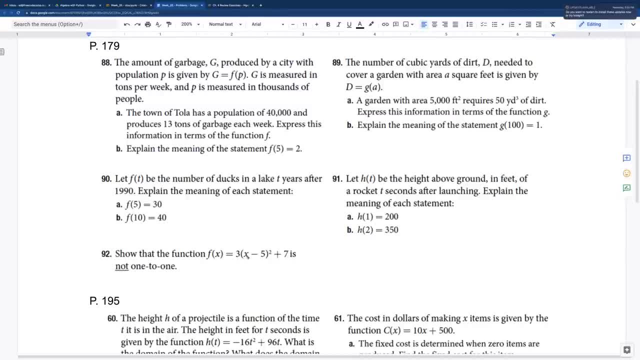 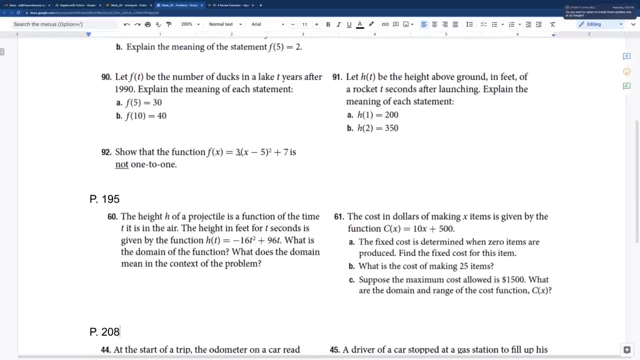 the 1 to 1, there's actually positive x values and negative x values that still have the same y value. So that's why it's just not 1 to 1, but it's still a function. I don't want to talk too much about that, we'll get to. 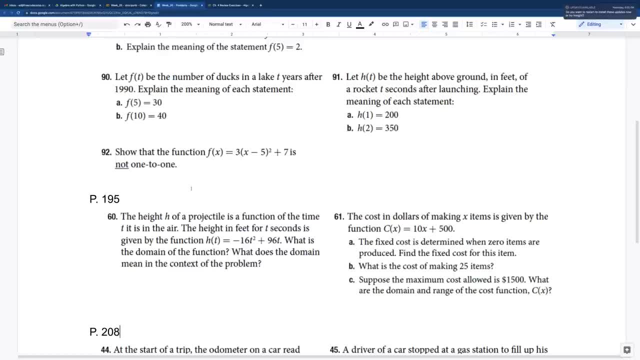 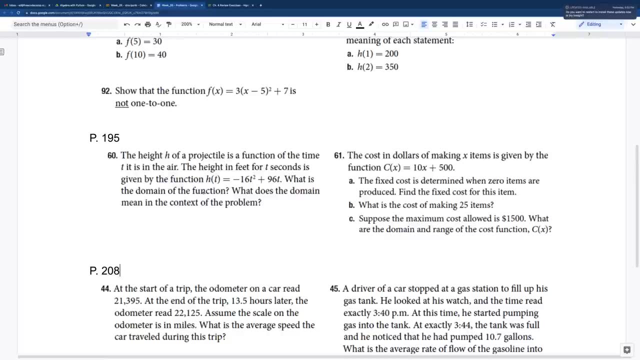 these types of functions later, but I just want to mention that in case you're looking at that and saying: well, what does this mean? 1 to 1?, So in number 60, now this is also not linear and you see the height of a projectile. 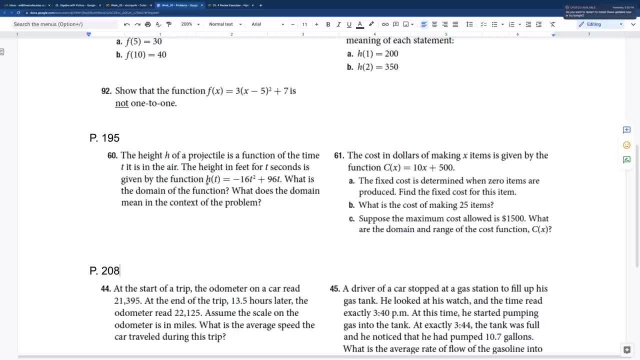 is more like something like this: After t seconds, here's the function: h of t: equals negative 16t squared plus 96t. So that's showing that you know it isn't linear. In fact it's a parabola, because it goes up. 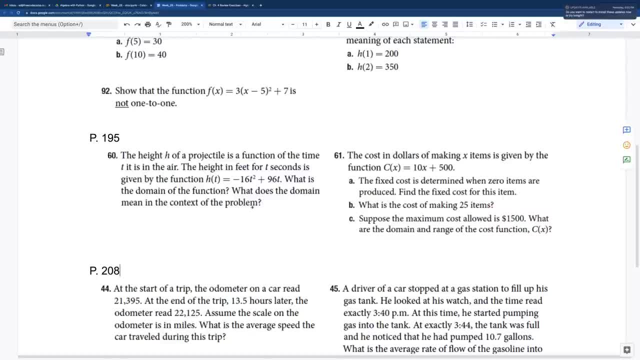 turns around, comes back down. Okay, So the domain: anytime we talk about the domain, that's the x values. So the domain is all the x values that are possible here, And then the range. this doesn't ask it, but the range is all the y values. 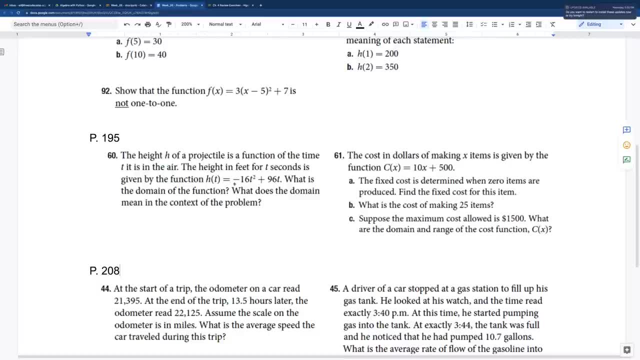 And this actually has a limited range. So, because this is a parabola that goes up and then comes back down, there's a maximum y value, So after that y value there's no more like. y values beyond that are not a part of the range, because 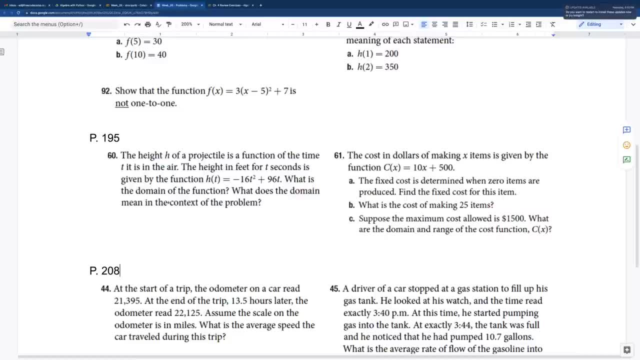 it'll just never get to those numbers. Then the domain: mathematically the domain is all real numbers, But realistically, in the context of the problem times, zero would be the first part of the domain. So you see. 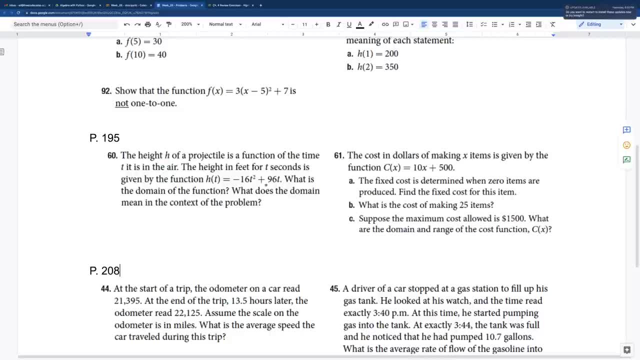 mathematically, these other numbers exist and they don't break this problem. But realistically, if I'm launching something, it starts at times zero And yes, I know that we can talk about t minus whatever and talk about negative values. 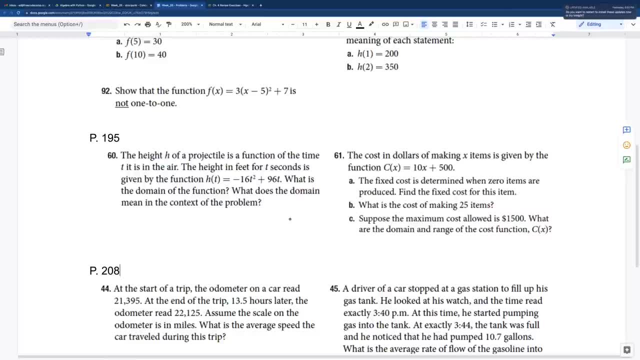 because we're awaiting the launch And this is second. so if it's like t minus ten, then it's, you know, t value is negative ten and that's ten seconds until the launch. But realistically we want this to be times zero And then the other one. 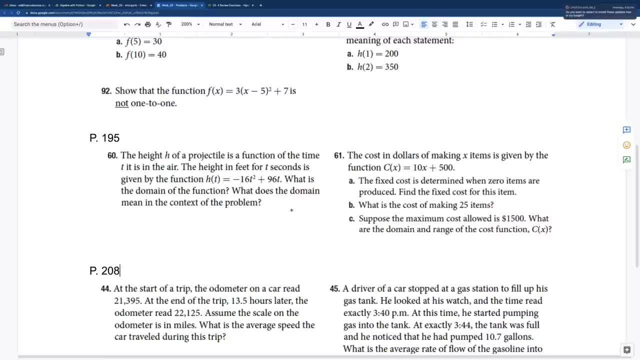 would be. it does go up and comes back down, So there's a time where it hits the ground again, And beyond that, it's not really within the scope of this problem. So let's take a look at how we can solve this. Just because, even though 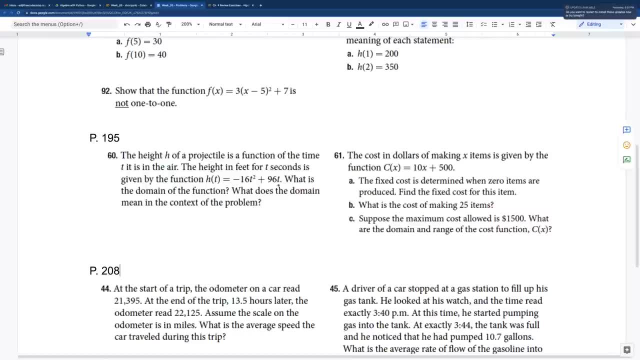 that's beyond what this is asking. I want to find out what that t value is. When does it come back down to the ground? Alright, so negative sixteen t plus ninety-six t. We can go into this where we're going to. 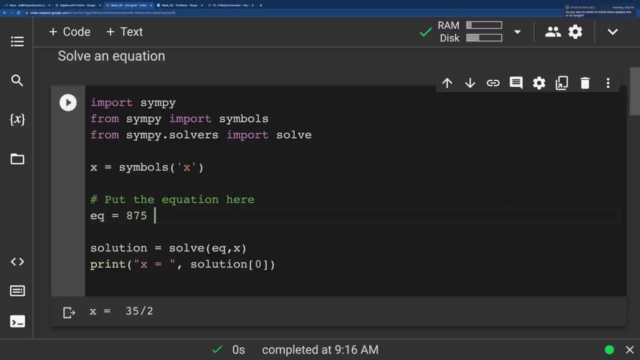 import our symbols And instead of t, we're going to make it x, just because I already have x as the symbol, Though you could always change it and make it t, That's fine. So negative sixteen, and again we're going to use x. 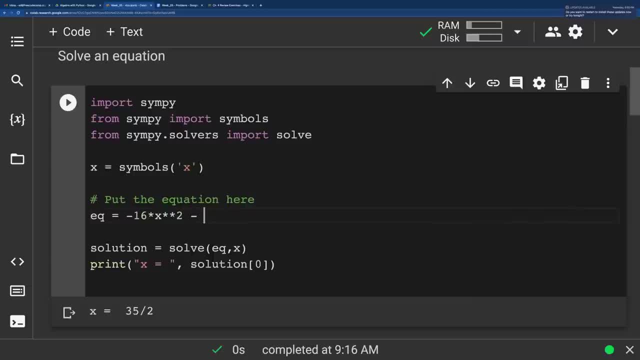 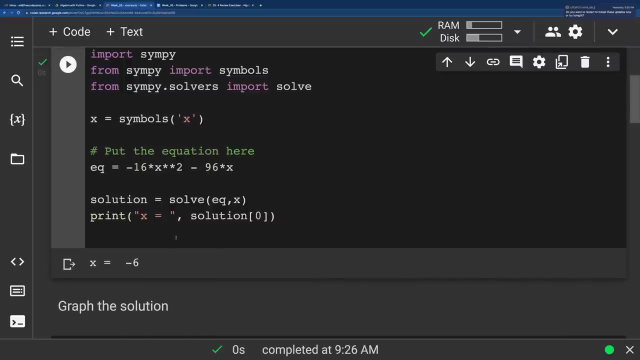 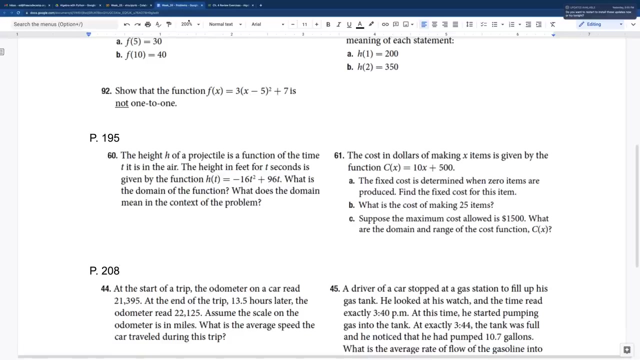 squared minus ninety-six x, And it's always- this is the equation- set equal to zero, and that's what I want. What x value makes this zero? Now, negative six would not be plus ninety-six t. Oh, because I put minus. 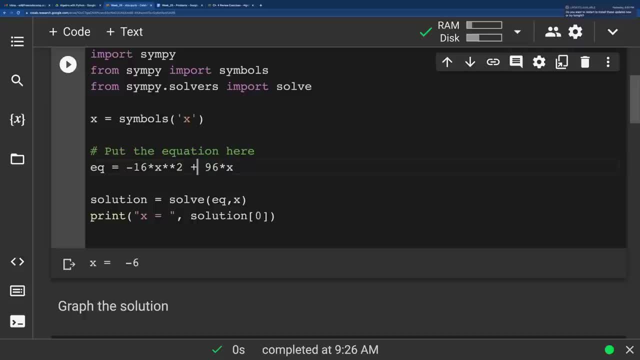 Yeah, Alright, So it only gives us zero? Um, what if I have? So I was doing this with things that only had one solution, so storing this as a finite set, and I just printed the first one, But this does have two solutions. 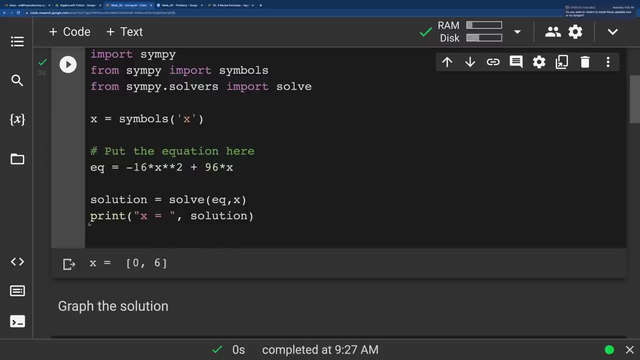 You see, And I mean I could get really fancy here and then actually just make another print statement. But see, this is my finite set. It's not zero, six as a coordinate, It's x equals zero or x equals six, And 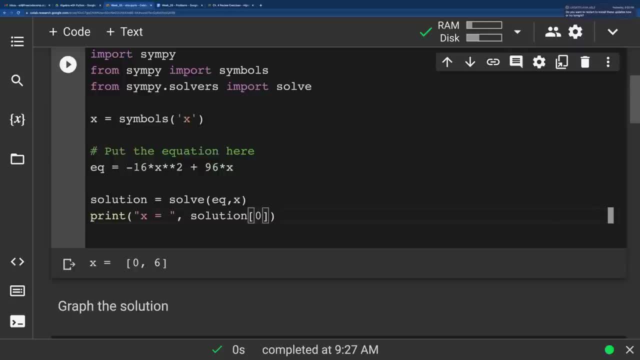 I could then put this zero and I could have another print statement. There we go To show the first one, And, but this is just a matter of you know how you want the output to look. And we have these, you know, we also have the, you know um. 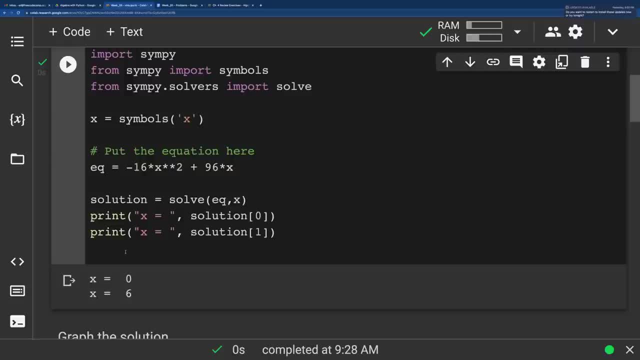 which we looked at before You. could, you know, loop through this Um to get solutions, to get multiple solutions? But there we go. Yes, x equals zero, It's on the ground, And then x equals six. 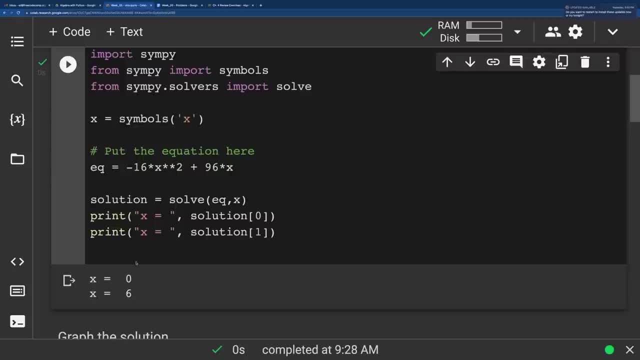 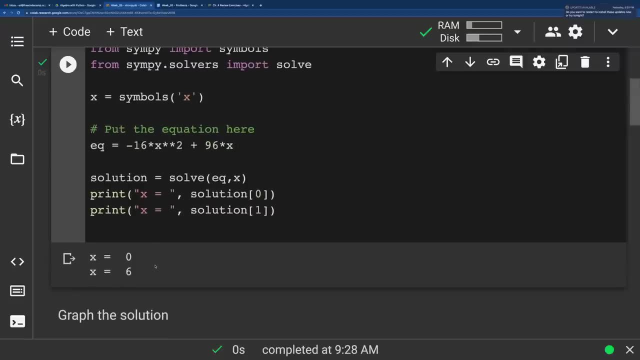 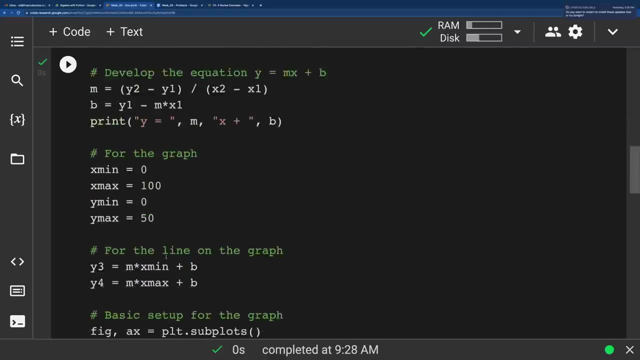 So that's another way that we could. you know that we could graph this Um, and we see that it's back on the ground at six. Now this is a little bit ahead, because we'll talk about quadratics later. So 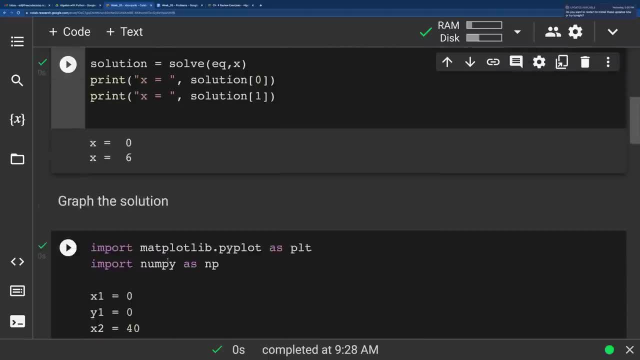 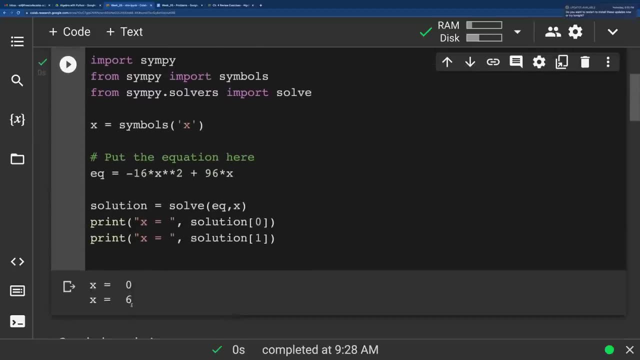 yes, we will. we will not worry about graphing this, because we'll get into this with quadratics, But this gives us the solution that at six um, at six seconds later, it's back on the ground. So some projectile. 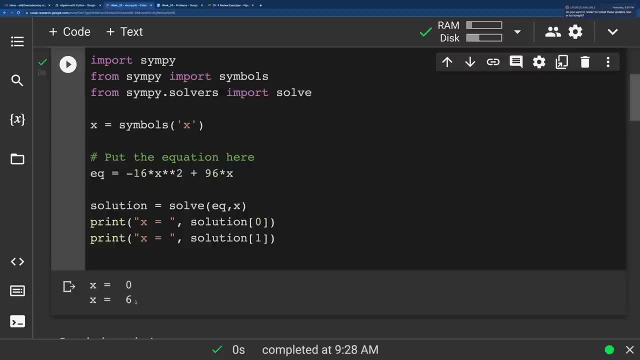 launched, it went up and turned And I'll tell you this that you know, halfway through these parabolas are symmetrical, so halfway through it's um, halfway through it's uh, at its maximum point. So 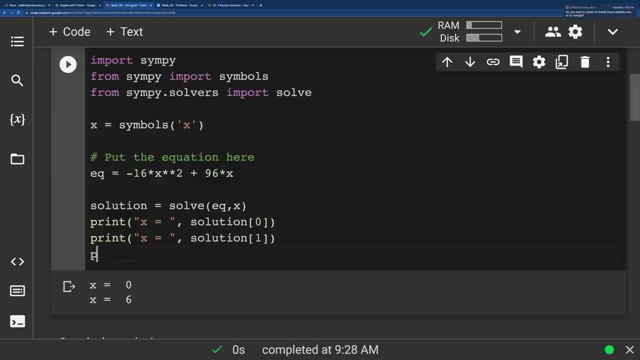 we could even print here what is that maximum point, and we can do that math: Um negative sixteen. here's what I'm gonna do, So halfway through that. so that would be three, would be x, And you see, that's really the idea that you know, we set up the. 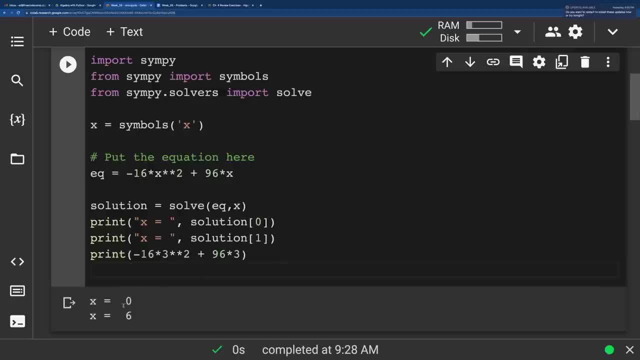 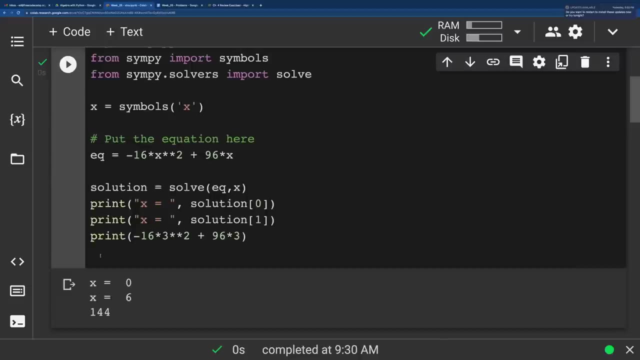 situation where I have x and then I can plug in my value. So zero six, it's back on the ground. So three seconds later it goes a hundred and forty-four feet up in the air. So realistically then, 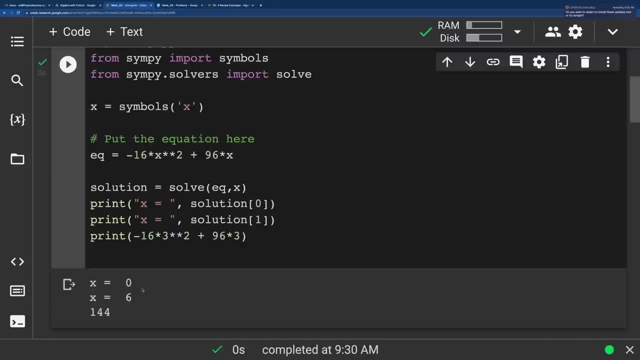 the domain for this function, as that that's practical, not just, like you know, mathematically it exists, but related to this situation, the. the only number, the only x values that mean anything for this are anywhere between zero and six, including zero and six. 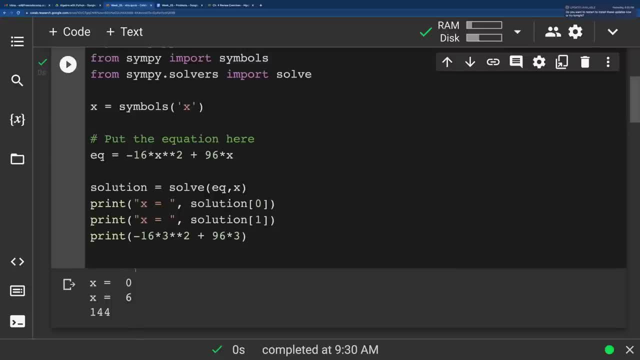 Because everything else doesn't really mean anything for this situation. You know, um, after this, then, if it keeps going down, like it doesn't go back down into the ground, And the y values here are between zero and one forty-four, So that's. 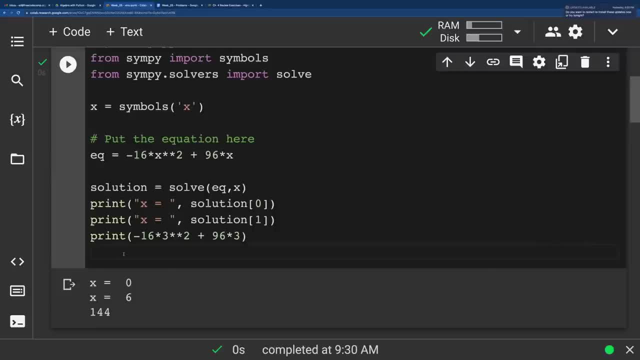 my domain, between zero and six, including both, and the range between zero and one forty-four. So you know these are some things we can look at. you know, solve When does it equal zero And plug in some various numbers. 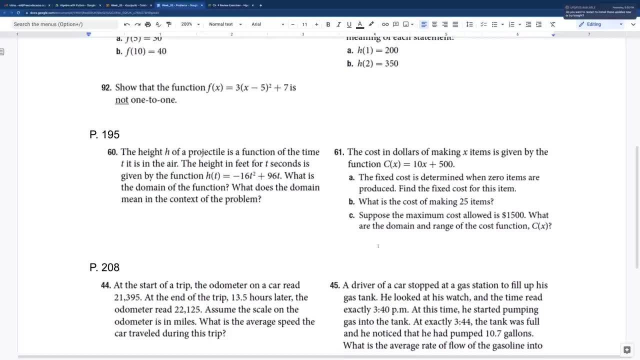 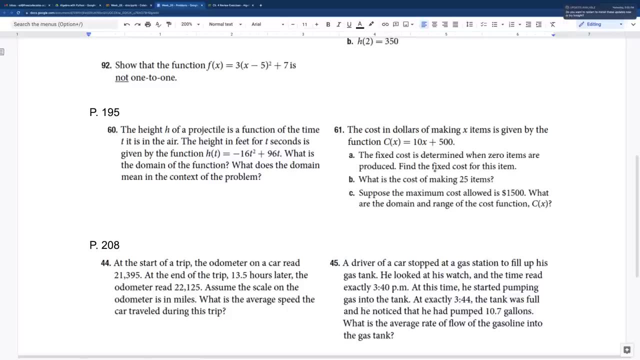 Alright. So if we look at sixty-one just again reading, reading these, these, we might not even need to do any code for this. We have this situation: the cost to making x items is ten x plus five hundred. 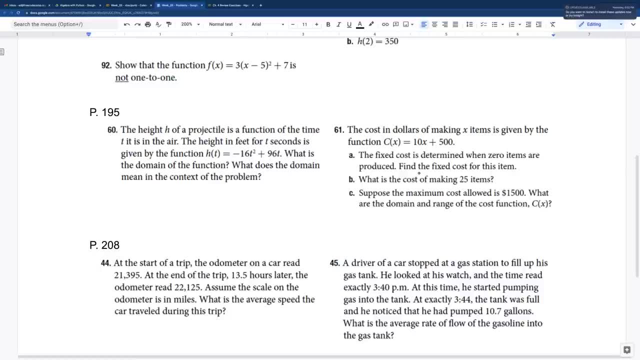 And the fixed cost is determined when zero items are produced. So find the fixed cost And remember zero. so then, if x is zero, that ten x drops out, and then we're left with five hundred. That's why it's b for begin. 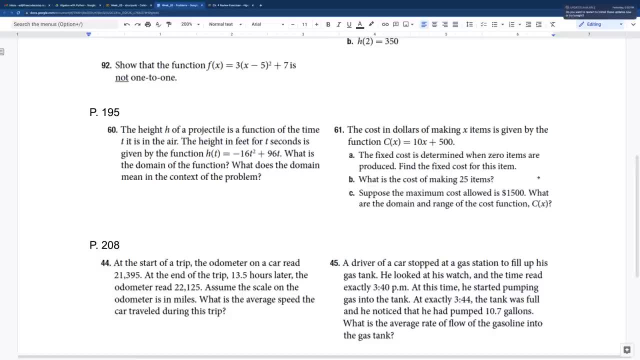 You know when, you know before we produce anything. you know the fixed costs are five hundred. Now maybe this is some sort of business and five hundred is like rent and utilities and everything that, even if they're there, they didn't make anything. 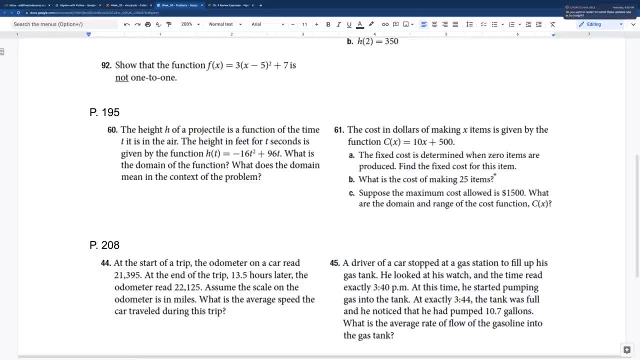 they still had to pay all that. And then they pay ten dollars for whatever you know, for whatever they're making. So then the cost of making twenty-five items would be ten times twenty-five. We would just plug that in Two hundred. 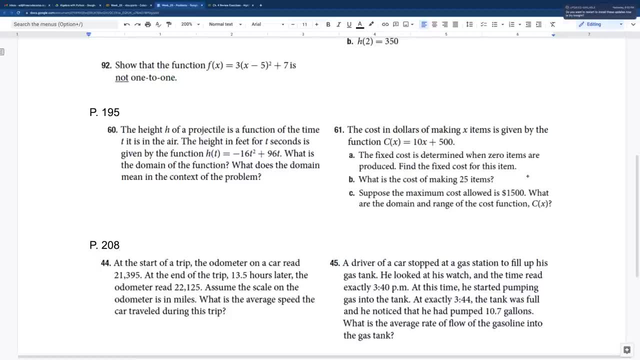 fifty plus five hundred is seven fifty. Alright, And supposing the maximum cost allowed is fifteen hundred, What is the domain in the range? So if we have to set this equal to fifteen hundred? Now, if we take a look at this and 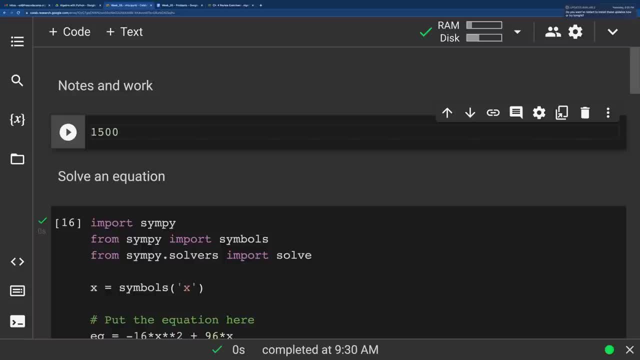 I'll just again write this here. So if we have fifteen hundred equals ten x plus five hundred- And notice, I'm not, this isn't Python syntax, because I'm not worried about doing anything with this yet- But then what do I want to do? 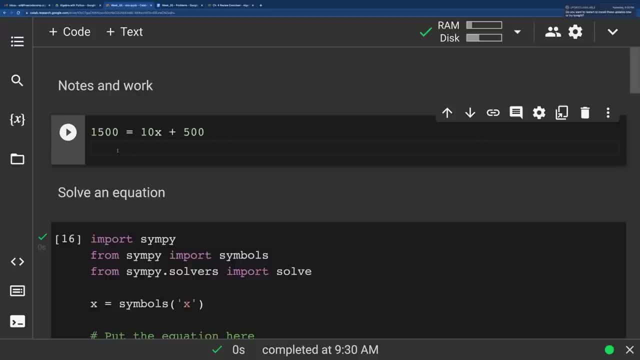 I want to put this equal to zero. so if I subtract fifteen hundred from both sides, then I get zero equals ten x minus a thousand. Because if I subtract fifteen hundred from both sides and so that's set equal to zero ten x minus. 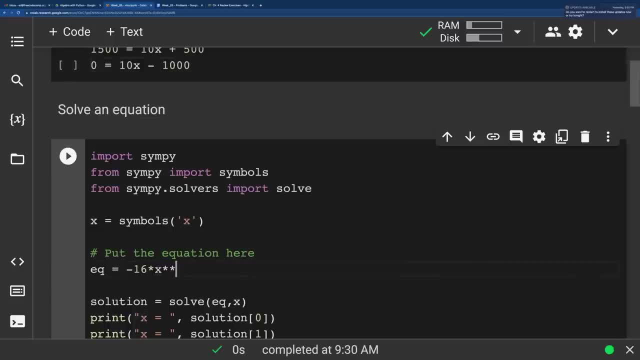 a thousand, then that's where I could plug this in here, So you see, you can work out the math before you get to the Python code. So ten and then here I do need ten x minus a thousand. So if that's the case, 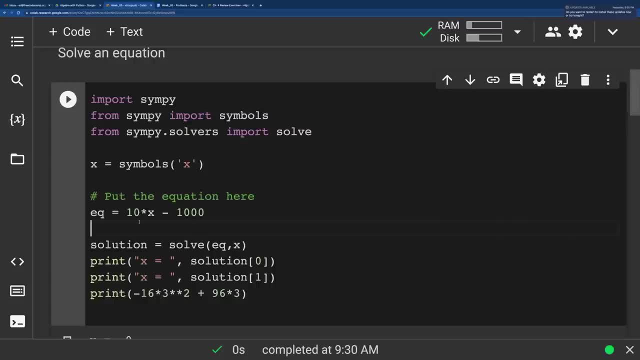 now with this one. I know there's only one solution, So if I keep the other one, that's going to give me an error. So, whatever it is, we know that we can only make a hundred Because, you know, maybe they only have that budget. 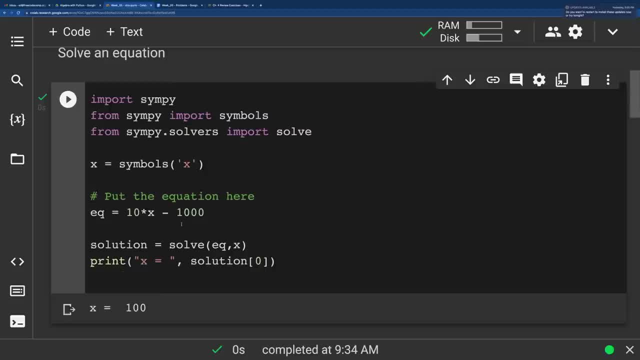 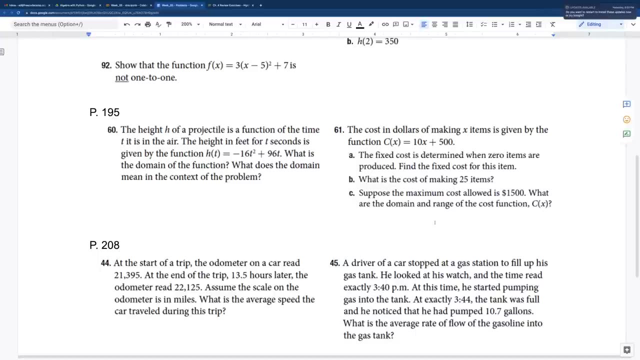 you know whatever they're making. they make a hundred of them. their total expenses were fifteen. total expenses were fifteen hundred. and then you know we have to go out and sell whatever they are. I don't know t-shirts. you know whatever else they're making. 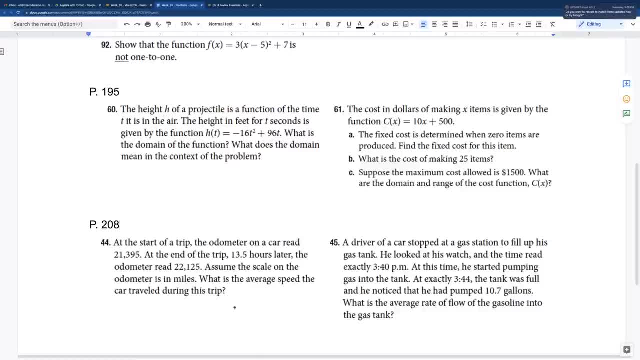 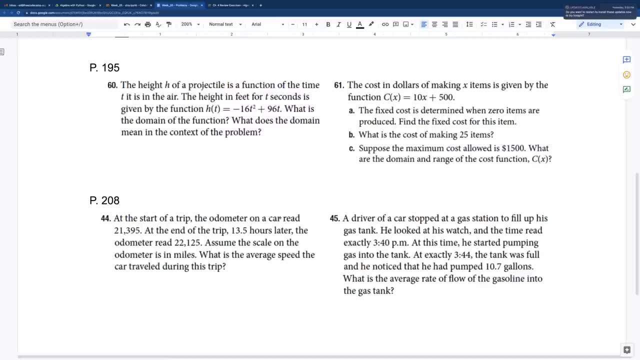 Alright, Okay so, and we see these same types of things. I just want to look at the setup of this: that at number forty-four, at the start of the trip, the odometer on a car read twenty-one thousand three ninety-five. at the end of the trip, thirteen. 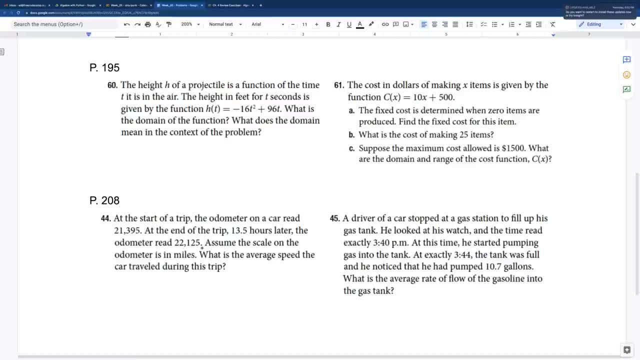 point. five hours later the odometer read twenty-two thousand one twenty-five. There we go, Assuming the scale is miles, So average speed. we want to take notice that anything like a rate like that, that slope. and we have two values: time zero and then the miles. 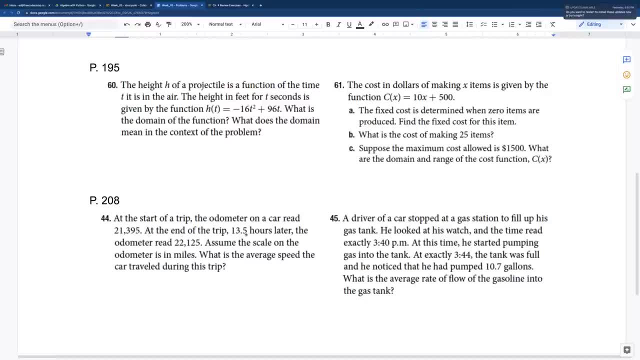 twenty-one, three, ninety-five and then time thirteen, point five, and then the miles, And we can go through and plug that in. whether I care about graphing this or not, it still will output the slope, which is the answer to this question, the average speed. 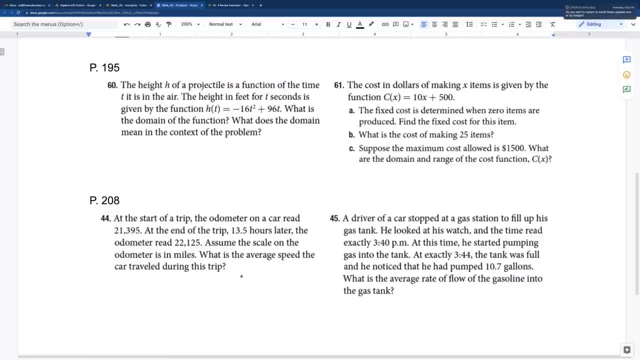 And that's where average speed, it would be a linear function, whereas realistically we know, especially over thirteen point five hours, the speeds going up and down, you know sometimes stopped, sometimes faster, sometimes slower, but we get that average speed. We know that, whatever that answer is, they're not going at that exact speed. 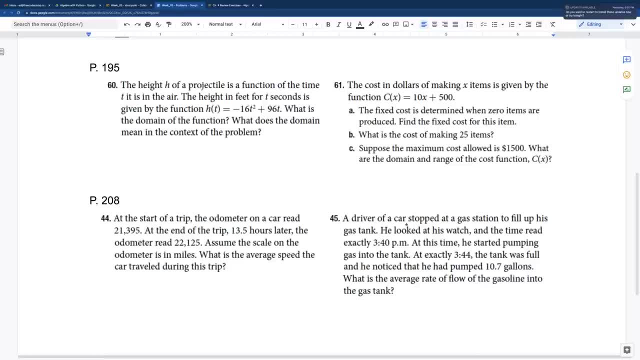 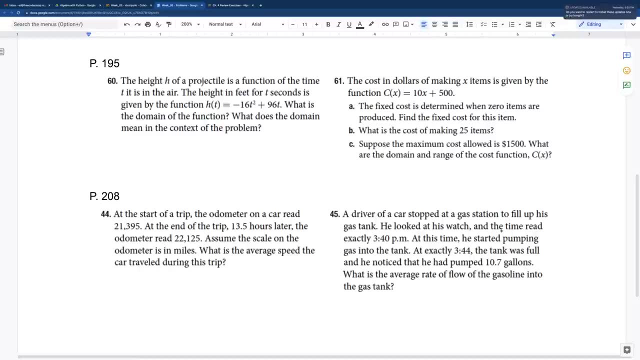 the entire time. Alright and forty-five. The driver stopped at the gas station to fill up his tank and he looked at his watch at the time and read: exactly three forty. This time he started pumping gas in the tank and exactly three. 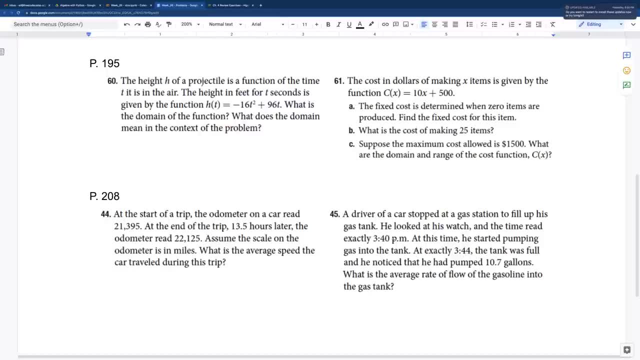 forty-four the tank was full. Now, if I was filling gas for four minutes, especially with these prices these days, I would be expecting it to be a lot more money. But he noticed he had pumped ten point seven gallons. So surprisingly, not that many, not that many gallons. 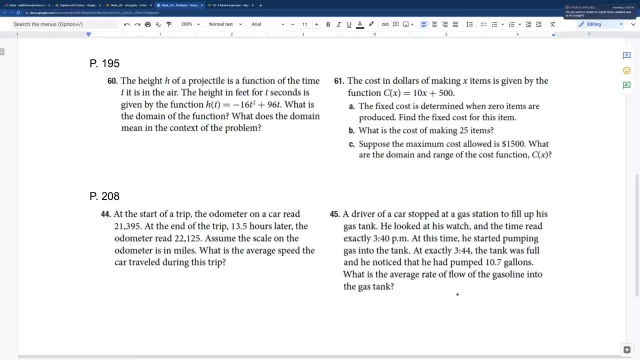 But what is the average rate of flow of the gasoline? So again, time is going to be x. so if we want to call it minutes, we can call it four minutes and then ten point seven gallons. So we could calculate to gallons per minute Or 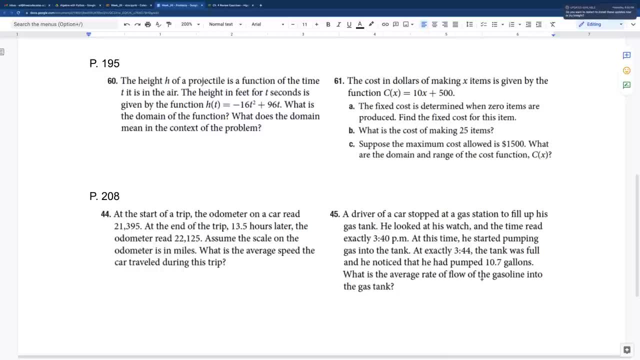 and again same thing. plug it in. Well, actually this one, because we already did that. subtraction is just ten point seven divided by four. So some of these, you know you have these scripts and everything available, but some of these, 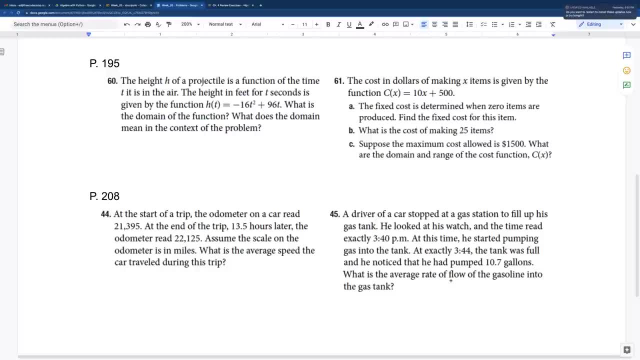 you might be able to solve even before you look at those. Or you could break it down into seconds- how many seconds in four minutes, and you know the rate of flow per second. But that's just. you know other possibilities. Gallons per minute is probably fine. 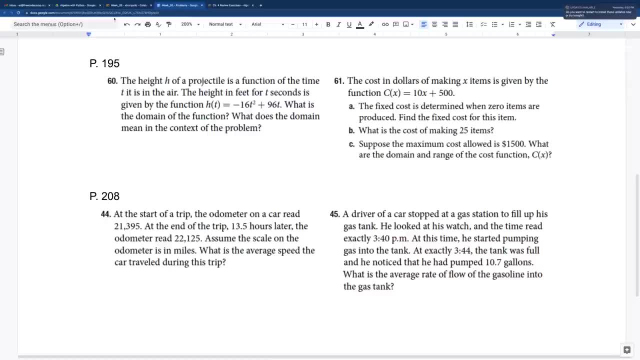 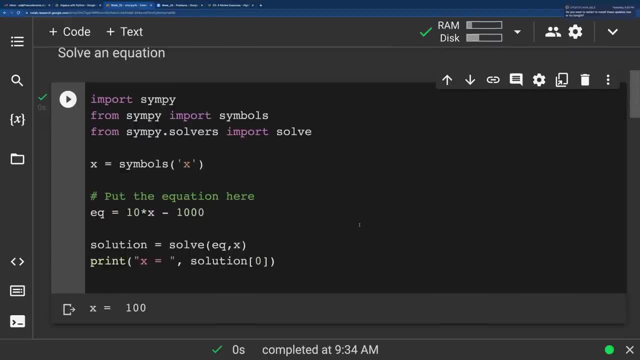 So we see all these situations. we want to see, like, recognize how we can set these up and the things that you're building, that you already have to be able to solve an equation, even if you know the equation is something else and you can just do one step. 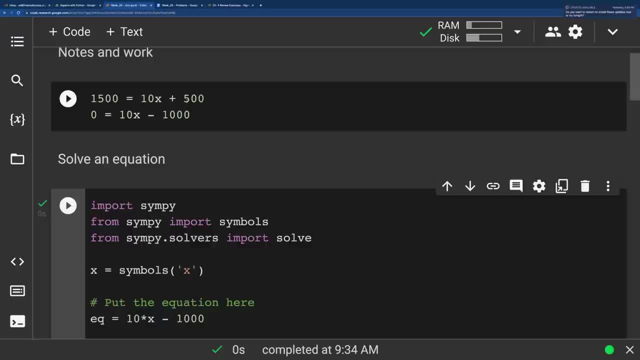 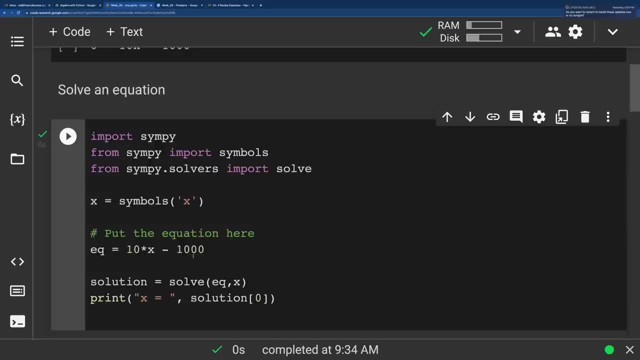 of algebra, you know, because that's it. you want to get it equal to zero. So, keeping in mind from earlier that one step of algebra, so then you have it equal to zero and you can solve it. So you'll have these things set up: solve any equation. 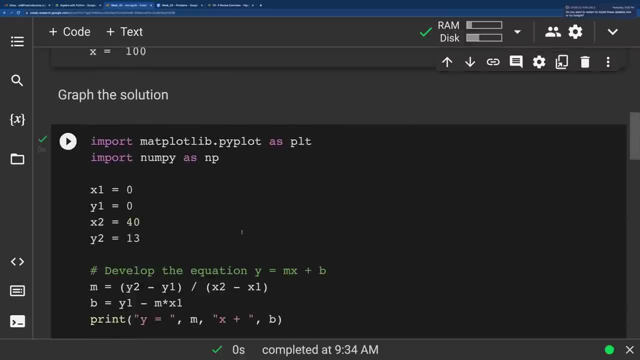 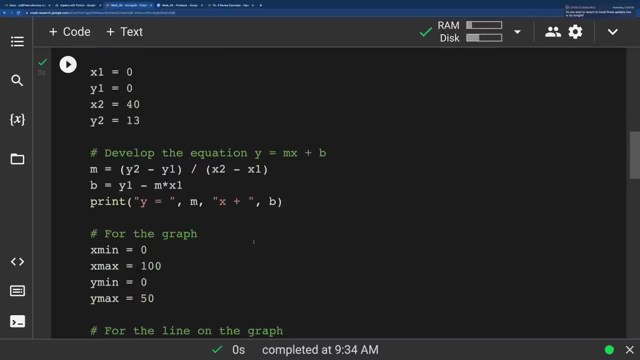 or you know, graph a solution, find the rate, all that. So you know, if all you needed was the rate, you know everything else here would be bonus, but it'll still also answer that question for you, So we want to see that you know. 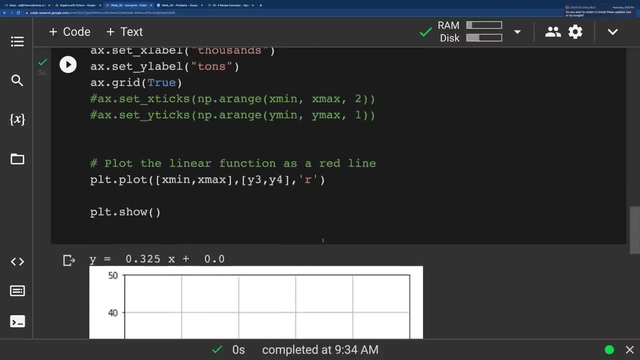 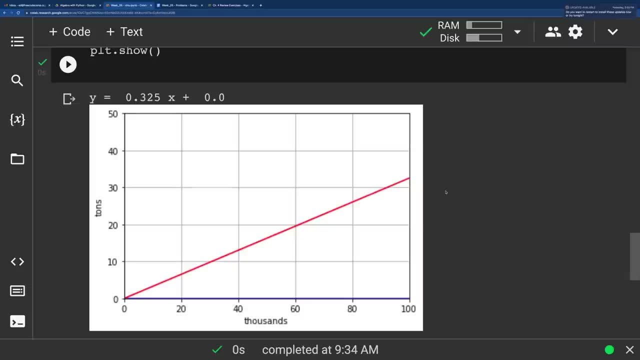 different ways that we can interpret these questions and solve the problems. graph them, take notice of some of the key words and hopefully you see how you can apply some of this to different situations that you come across. You know. look for situations in your day-to-day life and how you can apply these. 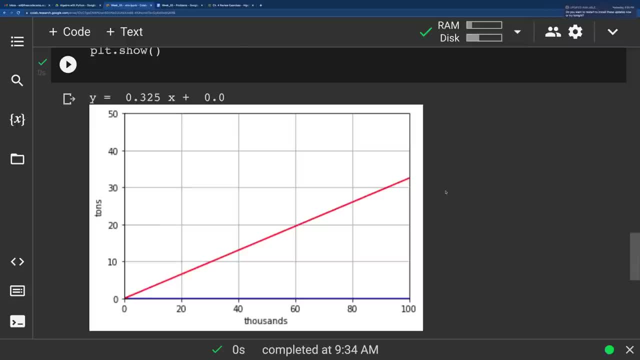 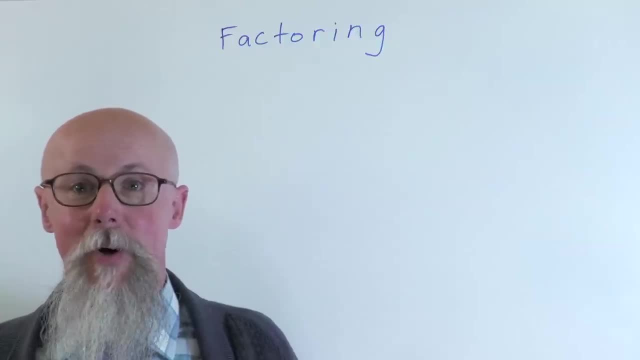 Alright, so hopefully that was pretty useful for you. So when we talk about factoring in algebra, then we're going to talk about dividing out something, So any factor is something that we're multiplying, And therefore I'm looking for things like when I see 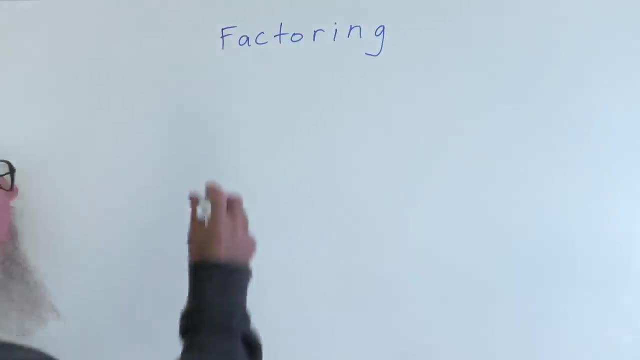 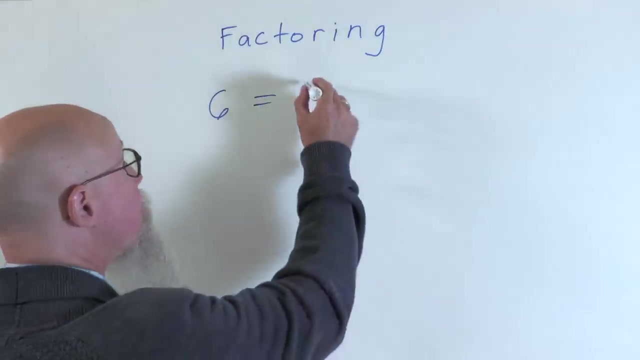 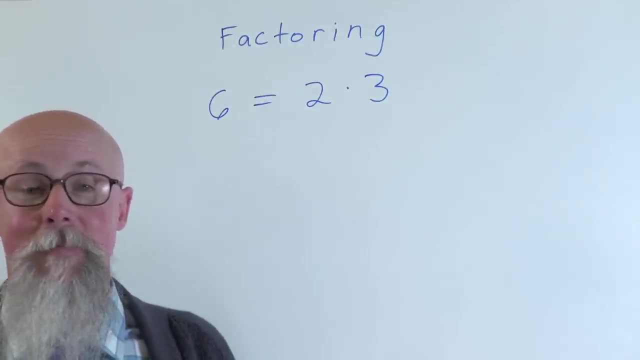 a number, what am I multiplying? So when I see a number like six, then I can say: oh, what are the factors? That's two times three. And here I'll put the dot for multiplying to separate the factors. So you know when I look. 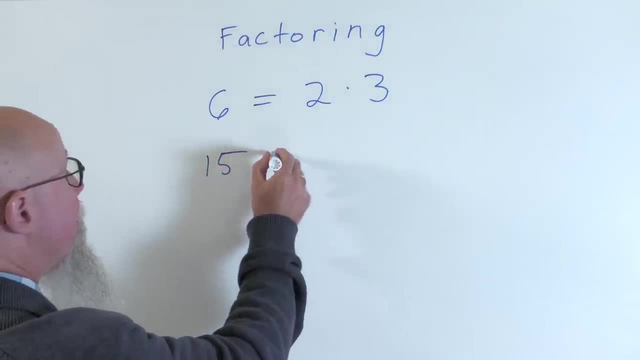 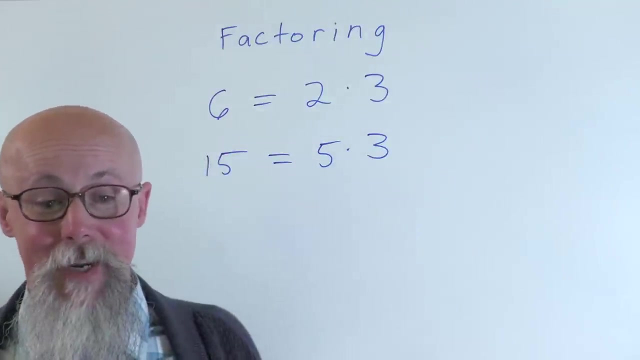 at a number you know, like fifteen, then what are the factors? Oh, that's five times three. And it's useful to be able to think about numbers and what are the factors, because that helps us reduce fractions and simplify other terms. So, for example, if 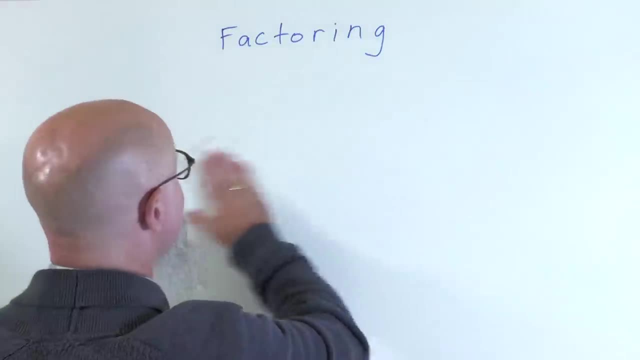 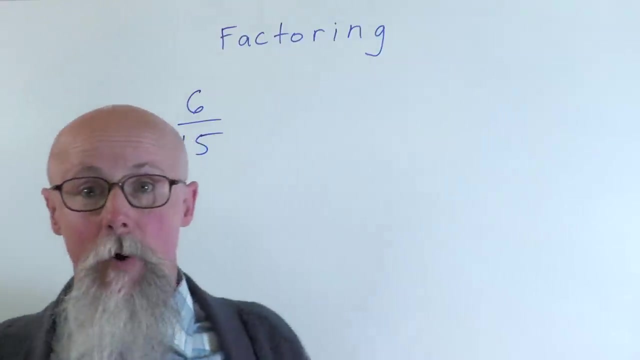 I had, since I'll use these two numbers here. supposing I had a fraction that was six out of fifteen And I said, oh well, I want to reduce that fraction to lowest terms. There's a better way to write this. 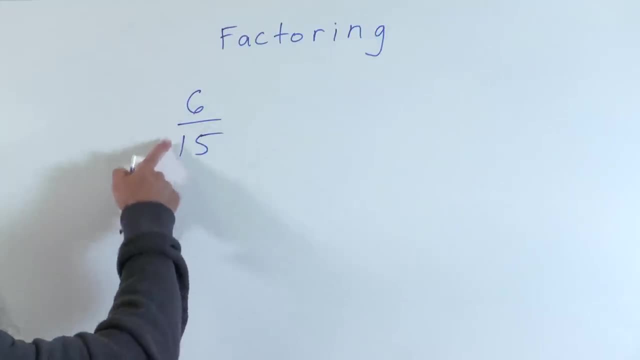 So then, if I remember that they both are divisible by three, that three is a factor of both of these, then I can say: six divided by three is two, and fifteen divided by three is five, And so this is that reduced fraction. 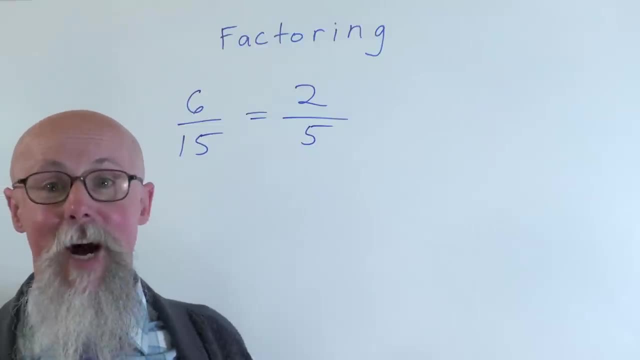 And I got this by factoring, I recognized the common factors and I divided out those common factors. So, just like other parts of algebra, if I do the same thing to the left side of the equal sign and the right, then it's still equal Here. 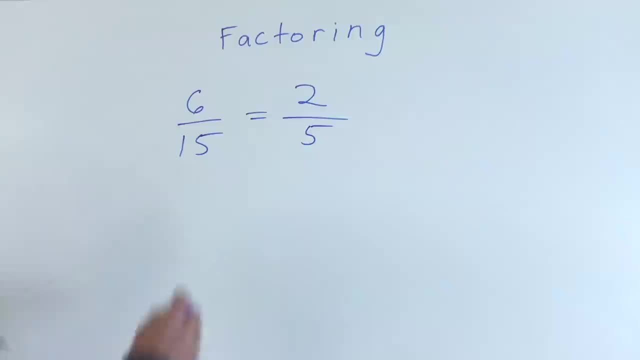 with a fraction if I do the same thing to the top as I do to the bottom. But that has to do with just multiplying and dividing. Adding or subtracting doesn't work. So if I have these, I can reduce my factors. I can. 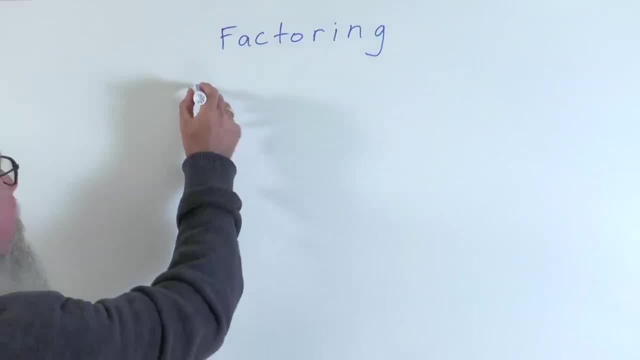 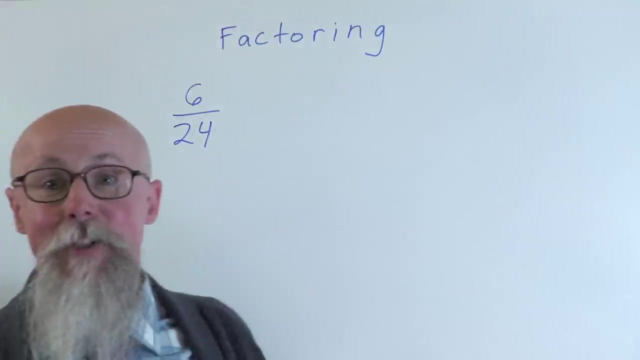 even keep going. Supposing I had something like six out of twenty-four, And supposing I didn't recognize that six was a factor of twenty-four, but I at least saw that they were both. even So, I could then divide by two. 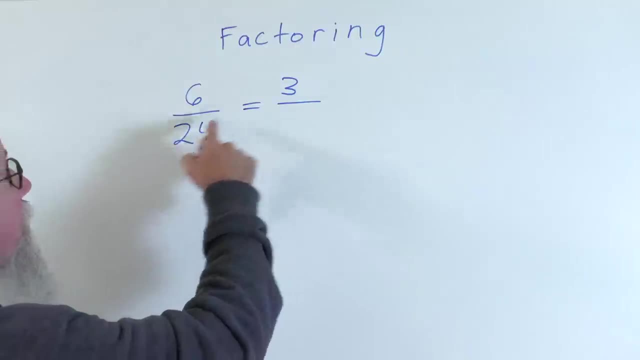 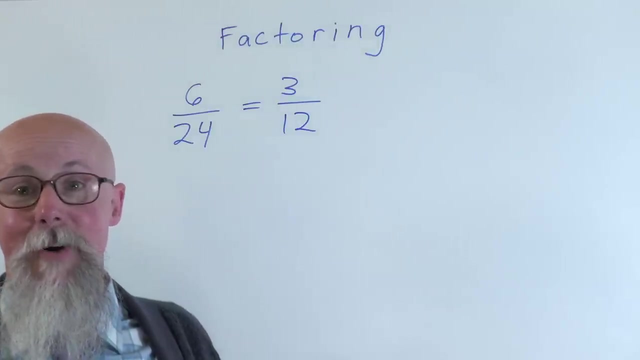 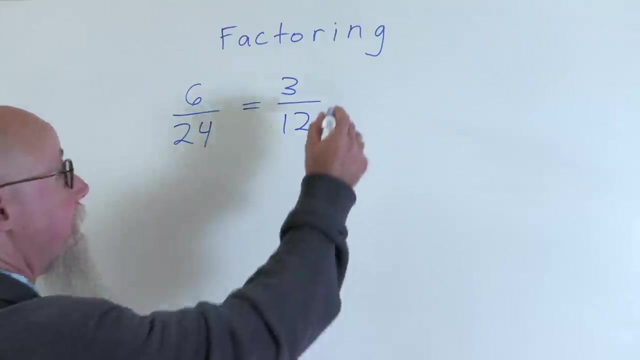 six divided by two is three. twenty-four divided by two is twelve. I could start reducing, again, recognizing that common factor. or then I could take it further: Oh, three and twelve, both divisible by three. And then I could say: three divided by three is one. 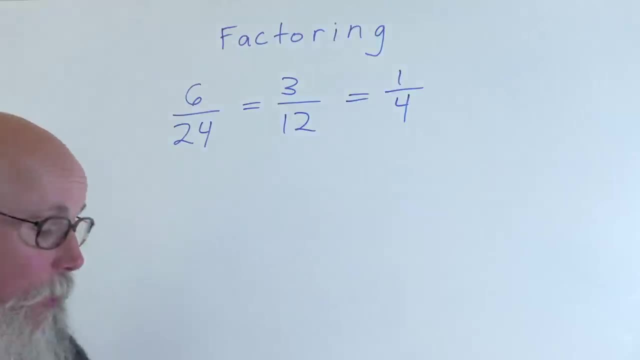 twelve divided by three is four. So again, I factored things out and therefore reduced the fraction. Now, a lot of times you know, we see things and we don't. we see fractions and we can't, you know, especially bigger numbers. 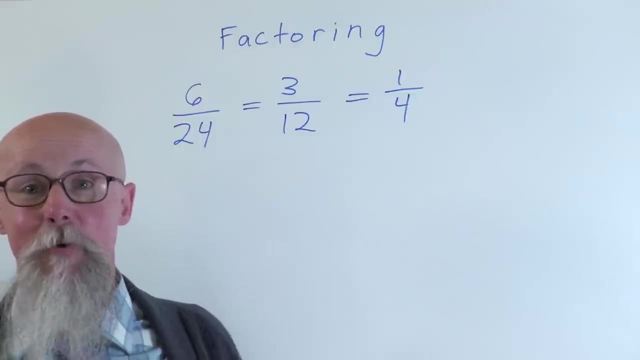 we don't right away think about the common factors, And we can always do long division. In a couple minutes I'll show you how to do this with code to set up a loop to find the common factors That way, even if you don't see them or if it's a lot- and you know how do I go through all these. 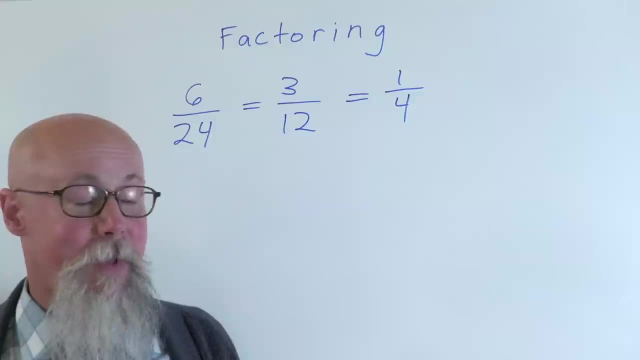 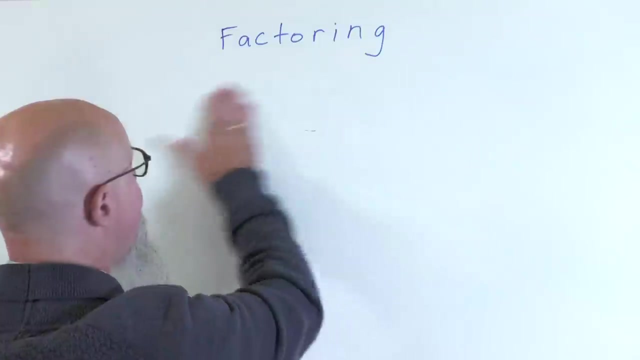 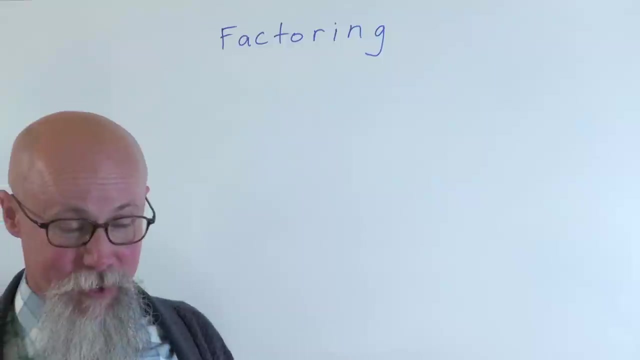 possible factors. I'll show you how to write the code to develop a loop to do that- find those common factors. But this is one of the big uses of common factors. Another use, and this is more related to other algebra topics: we might not need this as much as far as writing code, but if I 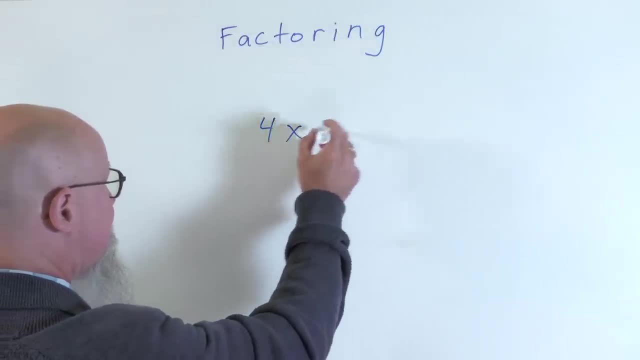 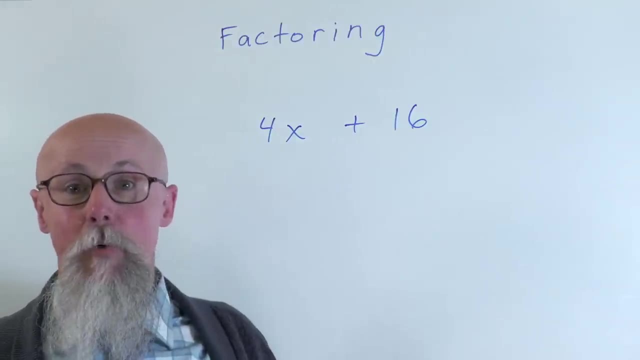 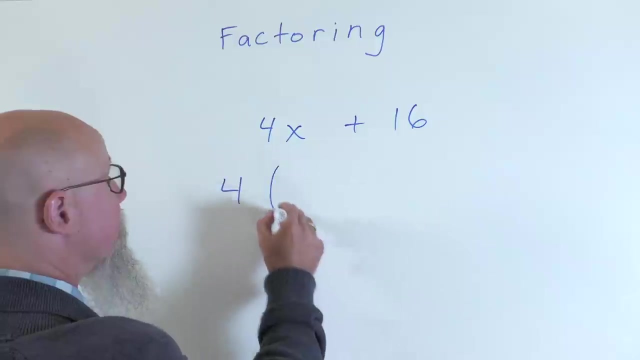 have something like you know, four x plus sixteen, something like that, and I say, oh, these two, the four and the sixteen, have a common factor, which is a four, and I can divide that out, and we can divide it out like this way. So this is another use of the word. 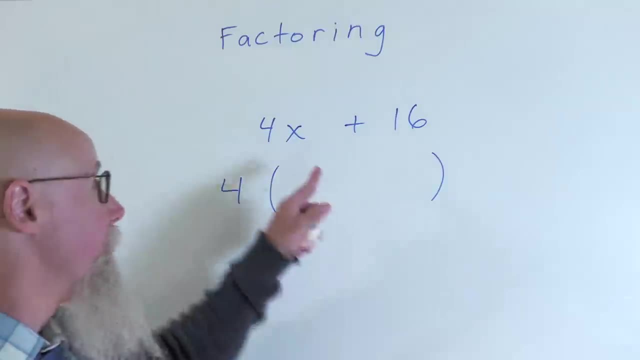 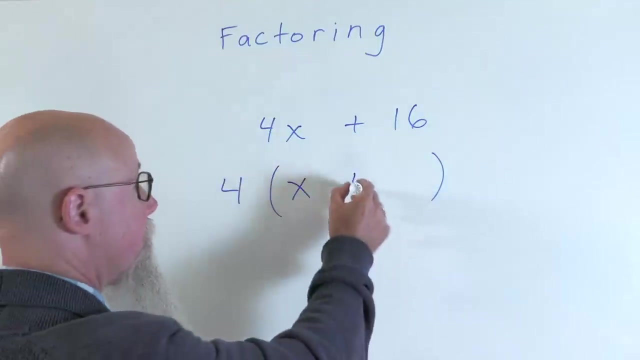 term factoring, because I see these common factors and I divide it out. Four x divided by four is one x, so I'll just put x, and then sixteen divided by four is four. So- and again this has more to do- 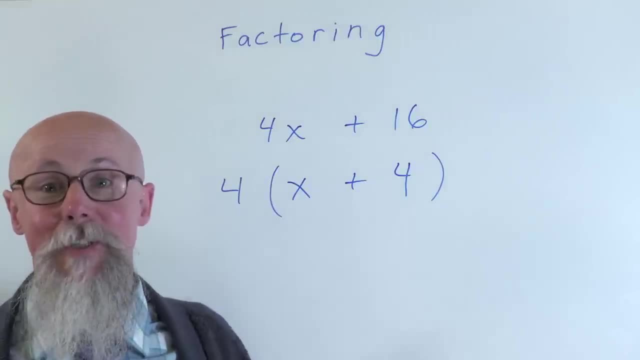 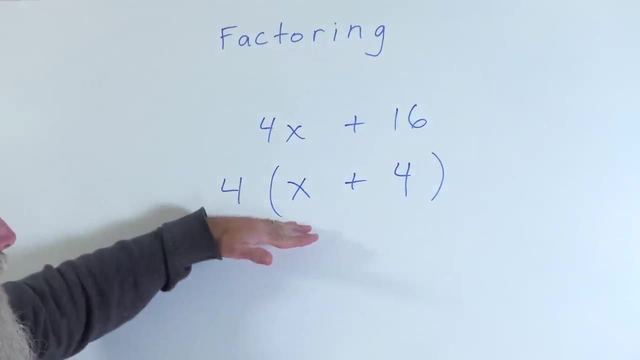 with other algebra applications. but I want to show you this because this is also factoring out. Then you know, if I have this, I see the common factor and I can divide it out and it looks like this, Or I can: 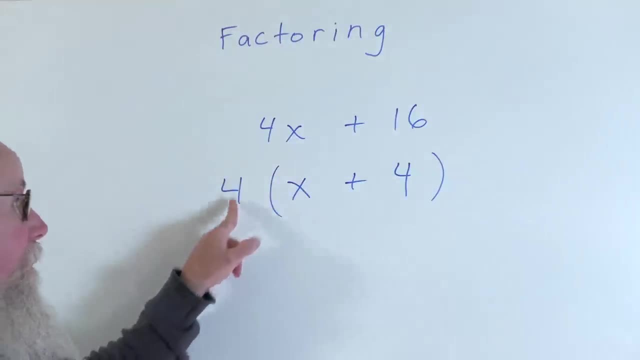 distribute the four: four times x is four, x four times four is sixteen, and get back to that. So that's another use of the common factor. One of the other things we're going to do is talk about factoring out square roots and 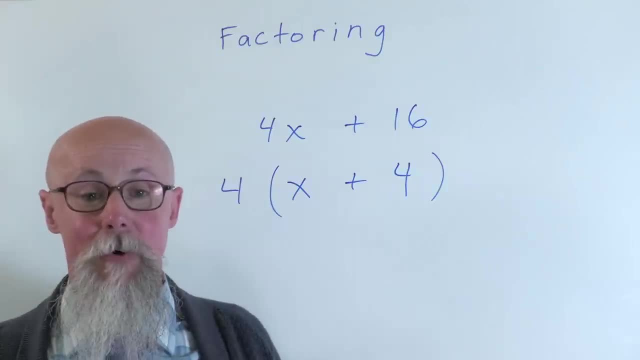 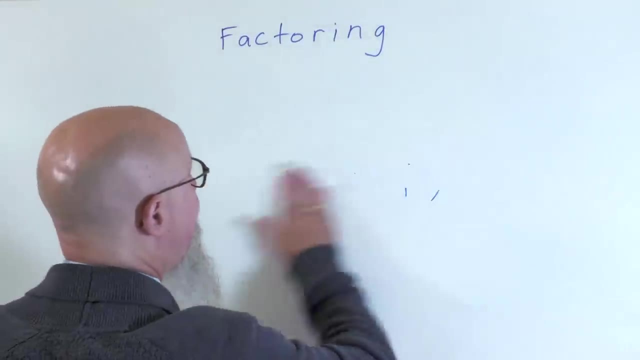 that also. I'm going to show you how to do this. but then we're going to look at the code. you know how to find common square factors and then factor them out. But let's take a look at this. If I have a square root, 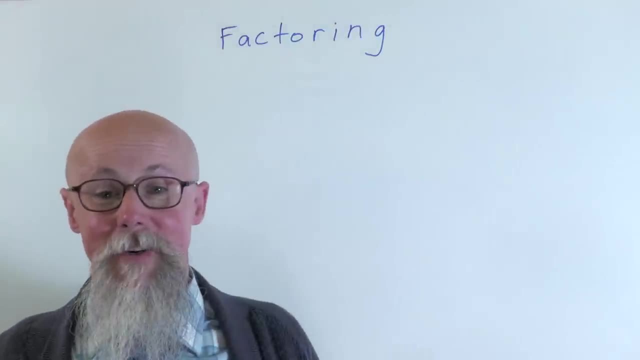 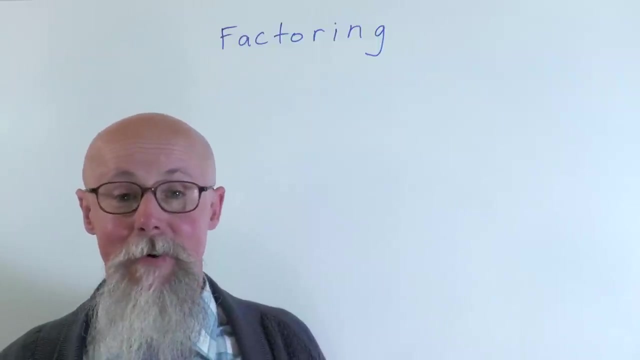 and sometimes we have square roots that don't work out evenly. they're not perfect squares, but I can factor them and sometimes that helps because those factors cancel out with other things later. So if I have, let's say, the square root, 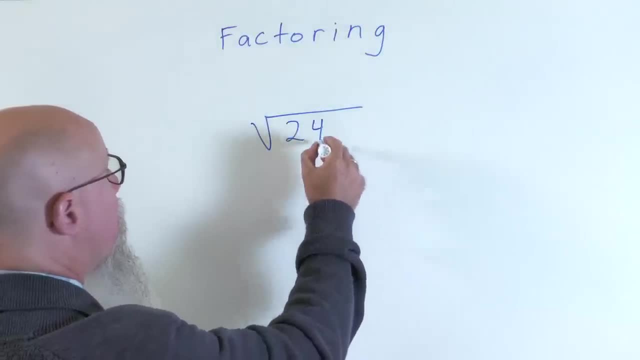 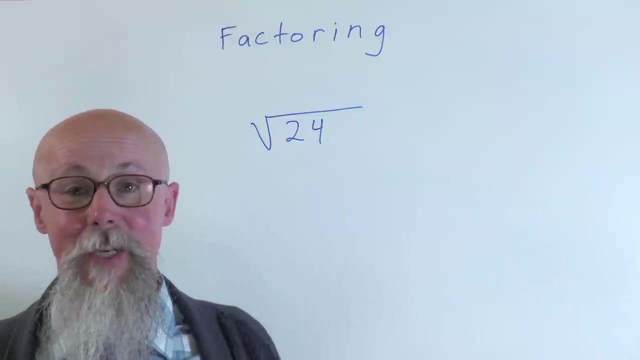 of twenty-four. Now, square root of twenty-five is five, that's great. Square root of twenty-four, almost five, It'll be some long decimal because it's an irrational number, But if I can factor that out, recognizing these common factors- and now in this case, I don't want just any factor, I want a square. 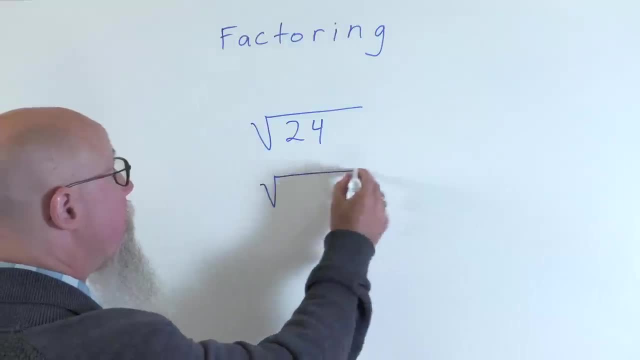 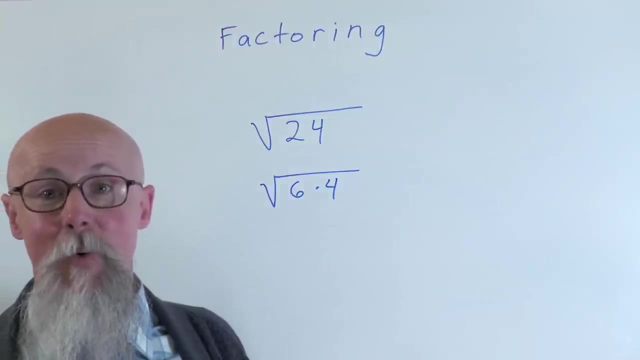 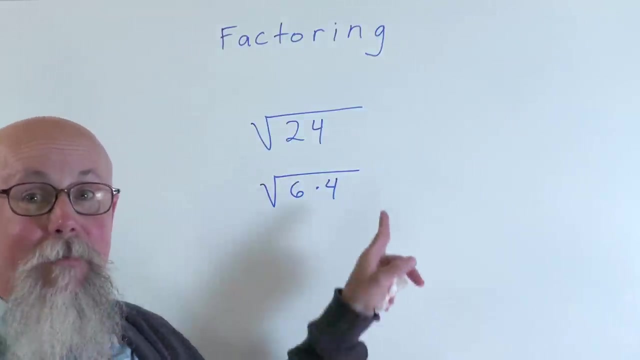 factor. So if I remember that twenty-four is six times four, that helps, because four is a perfect square And then I can say so. I want to identify these factors, but I'm interested in the ones that are square factors, and four is square, so the square. 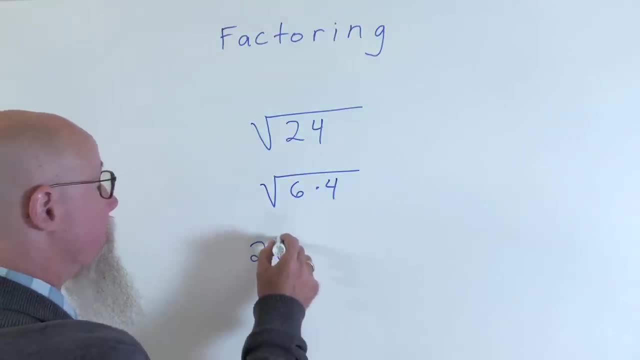 root of four is two, And then, since I took the square root of four, I still have that six underneath the radical. So even if I can't square root the whole number, I can square root part of it and factor that. 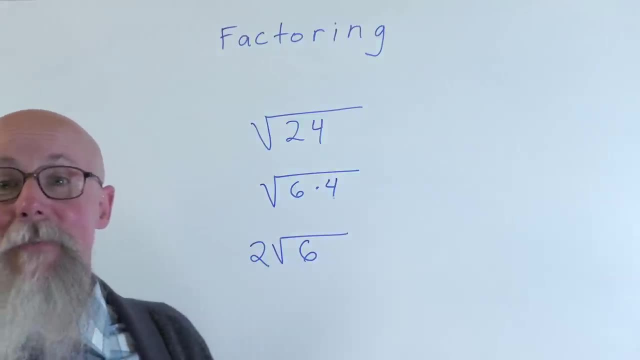 out. So sometimes then, even if I can't factor out something like the square root of twenty-four, I can get it down to something like this, and that's the simplified square root, this factored square root, and sometimes that's really useful. Now again, 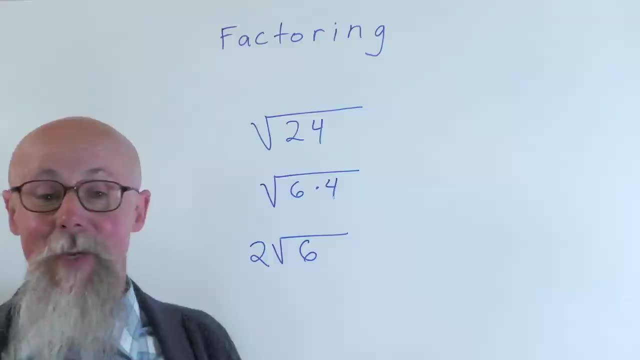 bigger numbers, things that you can't often think about. oh, is this a perfect square? We'll talk about how to write the code to find these perfect squares and divide them out, and even use the NumPy library to display it in a nice way. 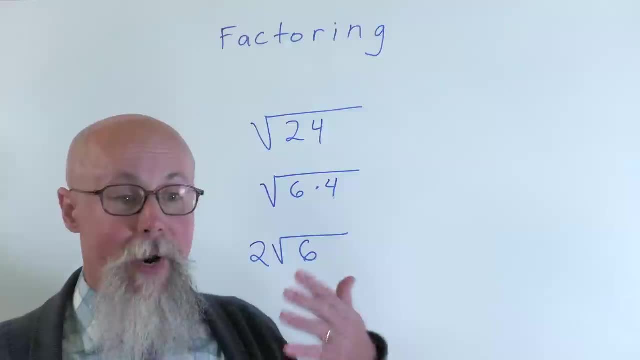 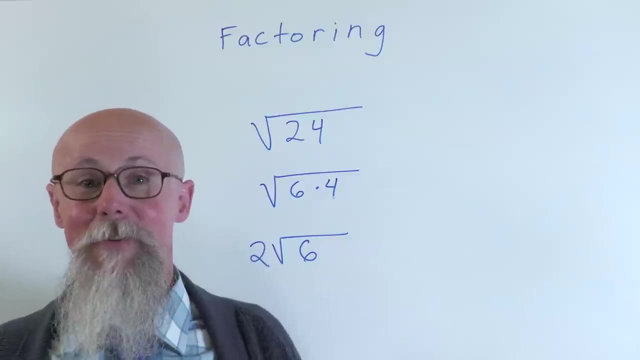 So that's really the essence of what we want to do with factoring, Recognizing factors of numbers, and this is where, even if you're going to write code, the more you remember your multiplication tables, the better things will be. It just makes things. 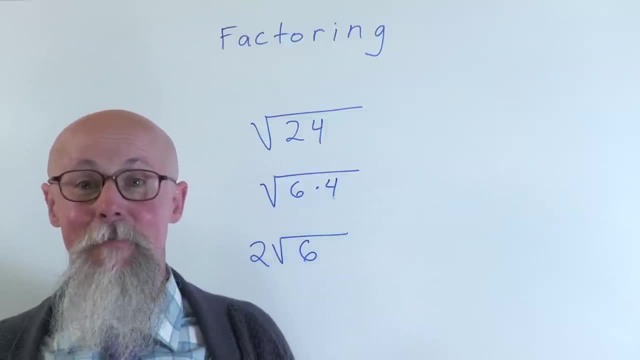 come together a little bit easier. But we're looking at numbers, thinking about what factors made that number, and then we're looking at common factors that we could possibly divide out, And so let's take a look at that. We'll take a look at the code. 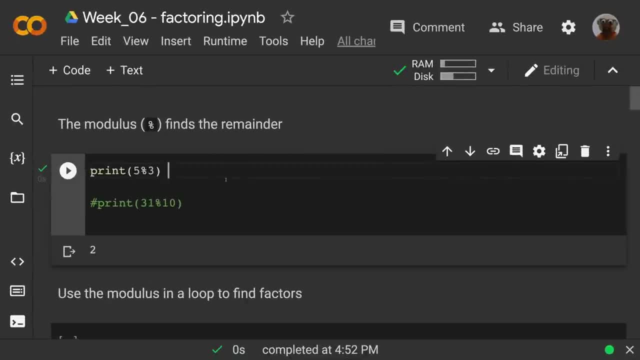 So here we're going to do the same thing we were doing with working it out by hand, finding the common factors, dividing them out- and it's going to work a lot better with writing code because it'll go through and easily find all the factors for you. 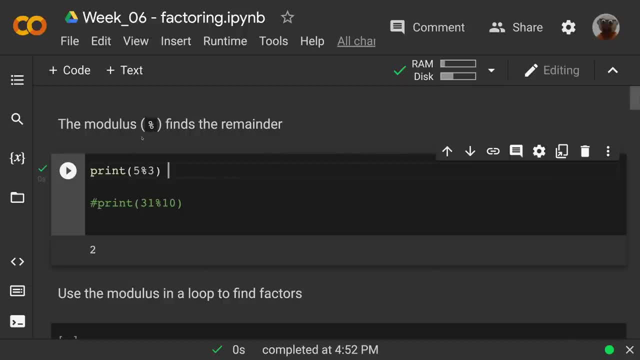 And to do that we're going to use the modulus operator. So modulus that is the percent symbol. so on the keyboard it's the shift on the 5 key. So what that does is that finds the remainder. So I already. 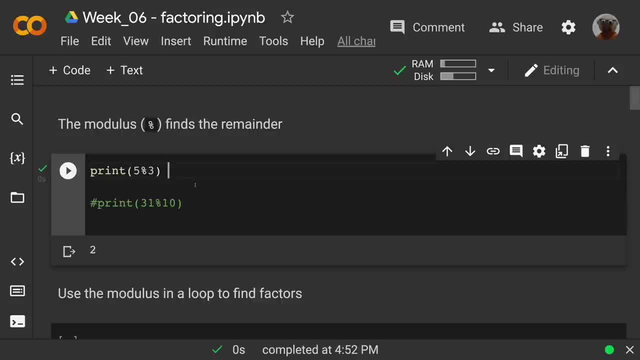 ran this. so if you print 5 modulus 3, it's like 5 divided by 3, but the whole number answer doesn't matter, We just want the remainder 5 divided by 3,. 3 goes in there once with. 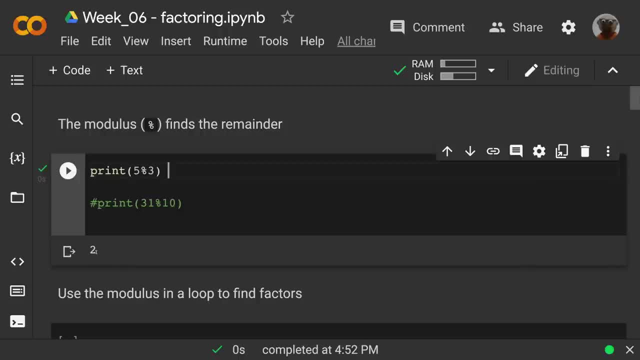 a remainder of 2, and that's what it'll print out- the 2.. And if we want, we'll just comment this one out and uncomment this, just to show you another one. So 31 modulus 10.. So 31 divided by 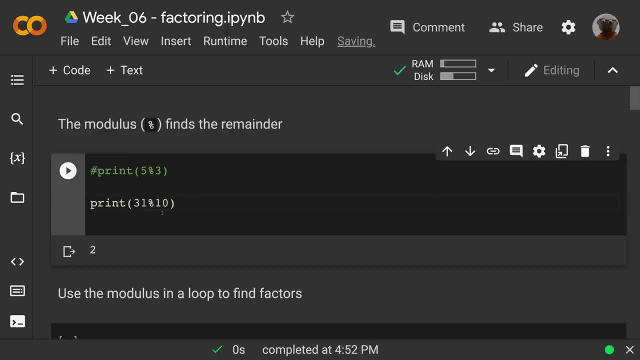 10 is 3, but that part doesn't matter. It's a remainder of 1, so when we run it it'll output 1.. Now, that's going to be important for finding factors, because a remainder means that the number's not. 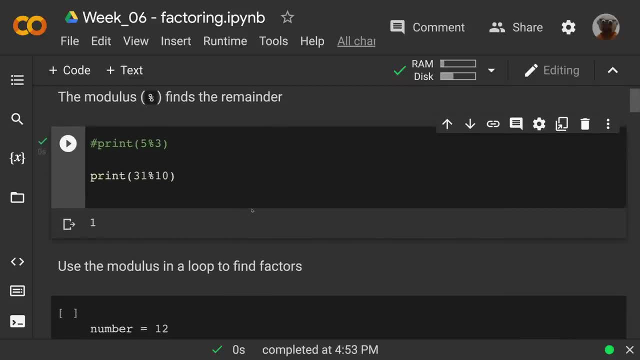 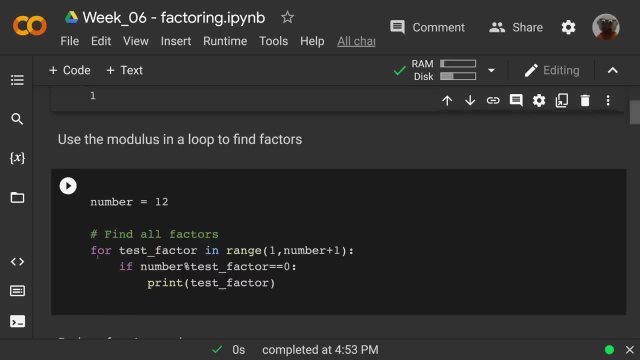 a factor, But if the remainder is 0, then it's a factor, and that's what we're going to do: Use the modulus to find factors. So I just picked this number, 12, and we're going to put this up. 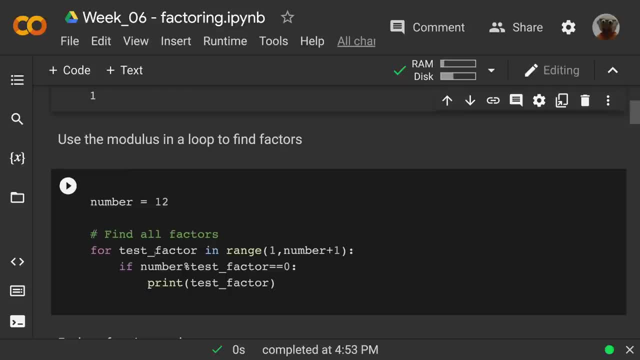 in a loop. So in our loop I made this variable just called test factor. So we have for test factor in range 1 to the number plus 1.. Because I'm dividing, so I have to make sure I start at 1.. If I start at 0, it'll give me an error. 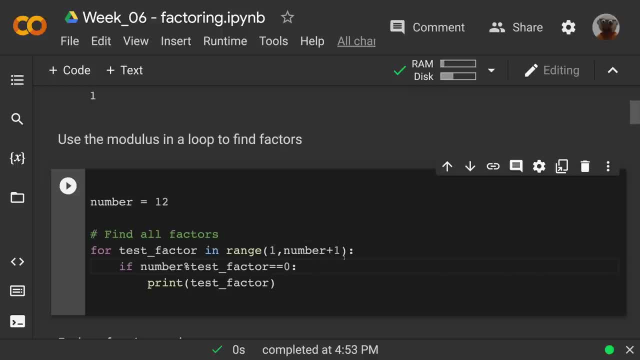 And I want to include that number itself. so I have to do plus 1.. Otherwise it won't do that last number. So for test factor in range, and then we go to this line here: If number modulus test factor is 0,. 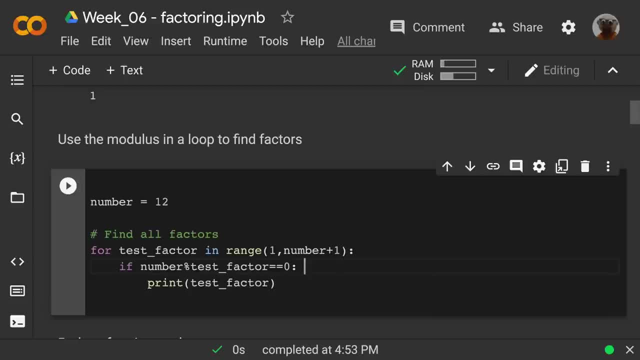 then it must be a factor. So then I'm just going to print out the test factor. So that's what this is going to do. Given my number 12 here, it's going to run through that and try each number. 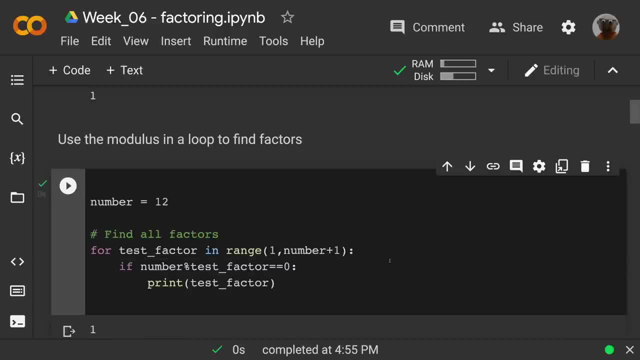 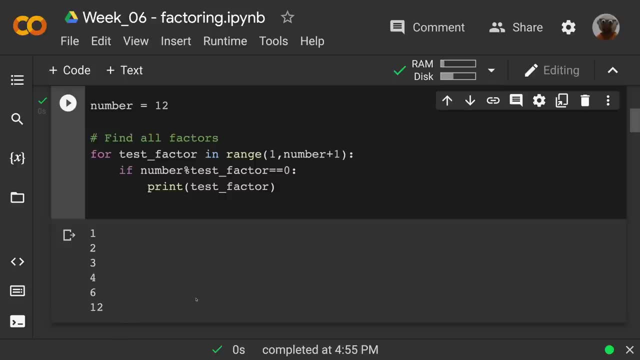 and see if it's a factor and print it out. if it is So, then when I run it see it prints. There we go: 1,, 2,, 3,, 4,, 6, and 12.. All of those are factors of 12.. 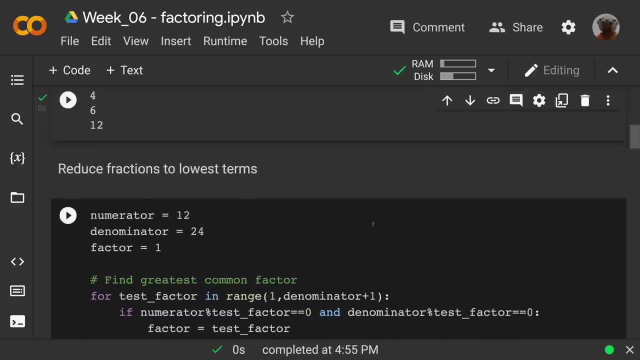 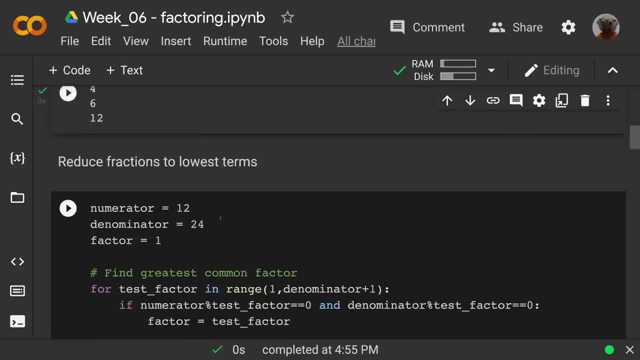 So how can I reduce fractions to lowest terms? So let's take a look at this, and I'm defining more variables here. My numerator, let's call it 12. Denominator 24. Now we know that this is going to reduce to 1 half and I'm going to define. 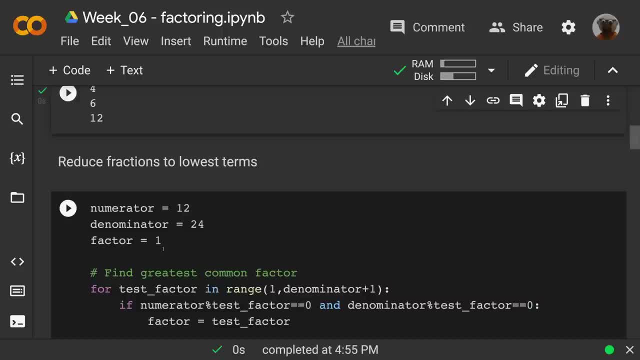 a variable called factor, which is 1.. That will be a factor and who knows, For some things that might be the greatest common factor. So now, once I have my numerator to find the greatest common factor, alright. so 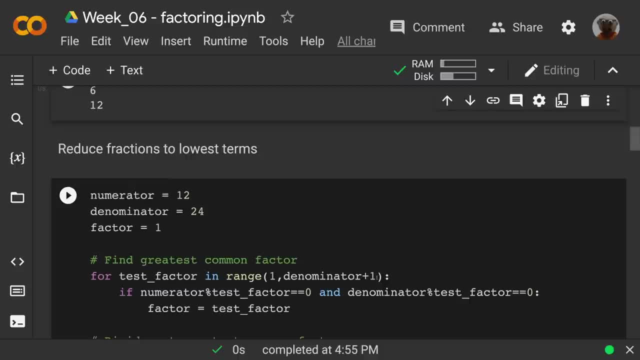 for test factor in range 1.. Denominator plus 1.. Because that's really it. I want to go up through everything in the denominator. Beyond that, the numerator is not going to really work out. So now, if the numerator so, we'll do this. 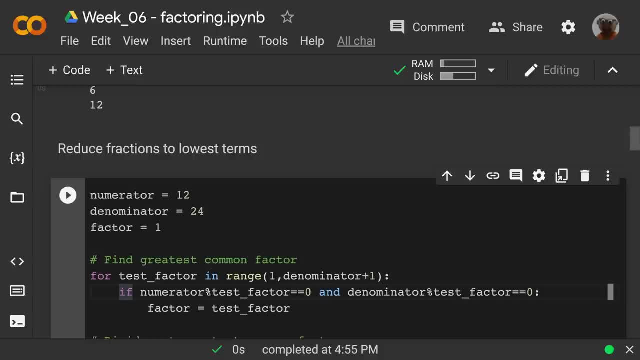 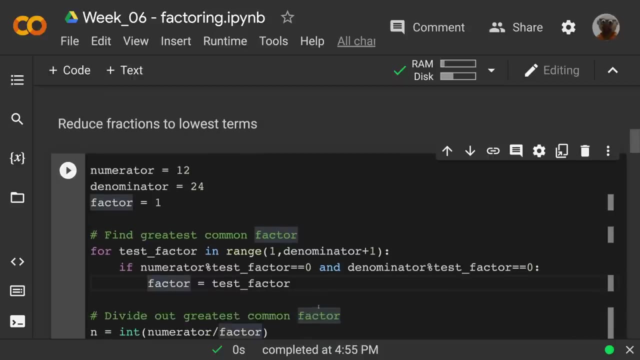 line here, if the numerator modulus test factor is 0, and denominator modulus test factor is 0. So for each of those, if it's a factor of numerator and denominator, now that's going to be my variable factor, And then, once I have that, 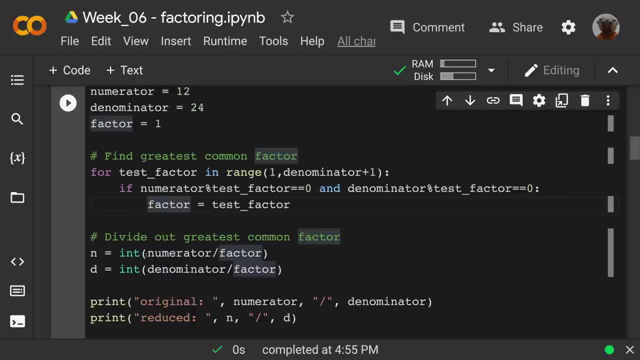 now I'm going to divide that out. So I'm going to do numerator divided by factor and I want to cast it as an integer because that's going to look nicer when we you know, the sense of this is that they should be integers if they're factors. 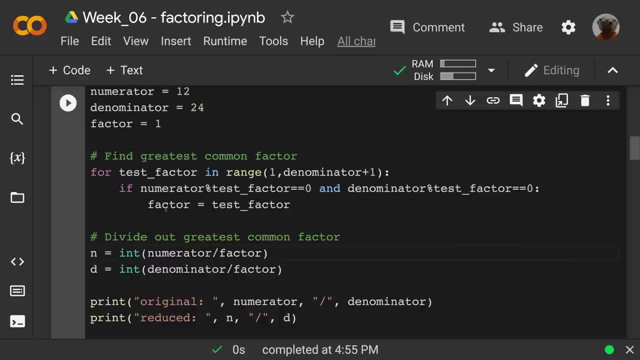 So this is going to look nicer when we display it. So once I find my factor and you know it could stay at 1, or it's going to get you know the largest factor I can find Once I find that. 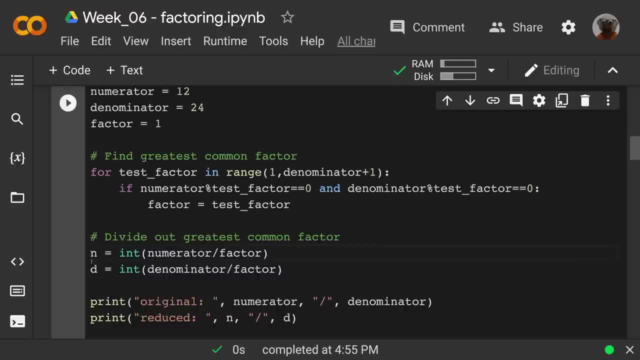 numerator divided by factor cast as an integer, and I'll just call it n- Denominator divided by that factor cast as an integer, I'll call it d, And then we're going to print out the original numerator divided by denominator, and then 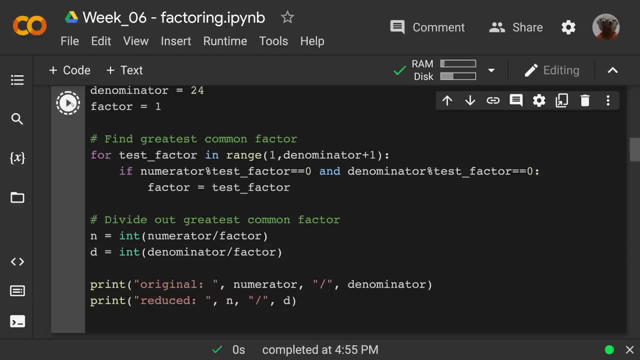 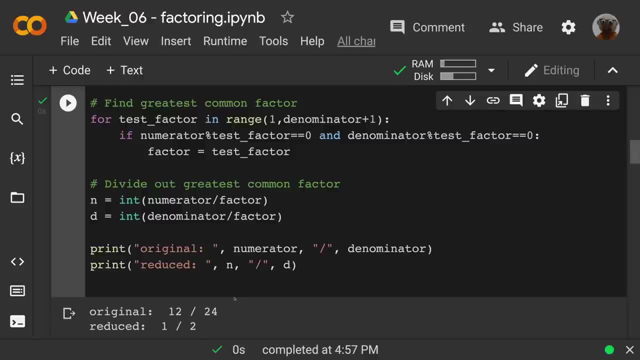 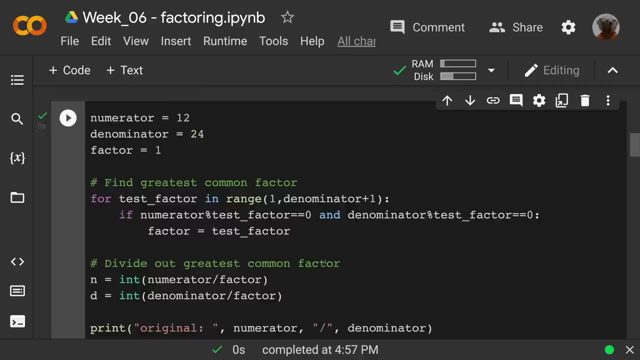 the reduced fraction n divided by d. So let's run this and we see that the original was 12 over 24, and the reduced is 1 half. So there we go, We can reduce any fraction, and you can even copy this code. 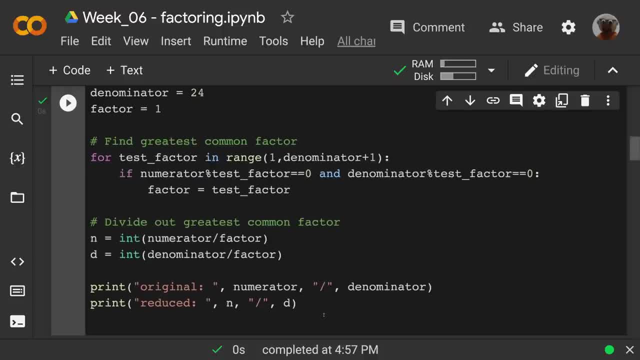 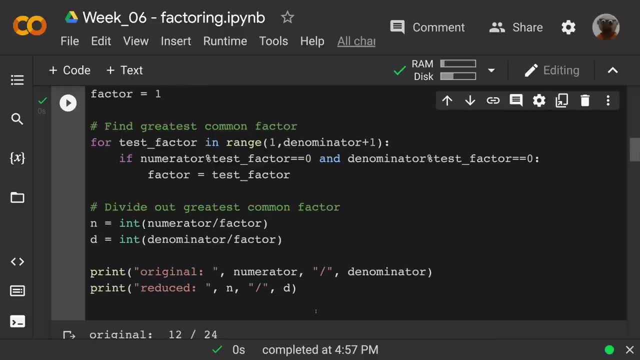 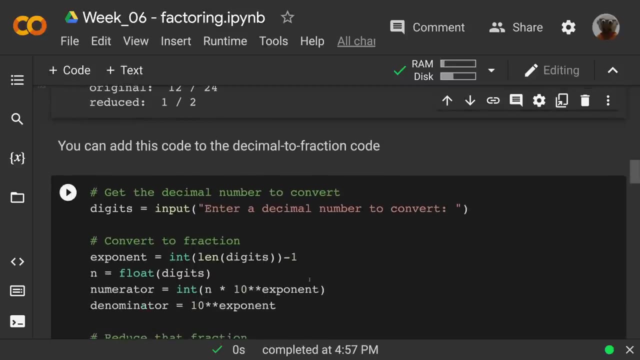 and use it within something else you have, or you can put this as its own function and deal with it that way. We'll talk about creating functions out of a lot of this code later on in the course. So the first thing I mentioned about adding it. 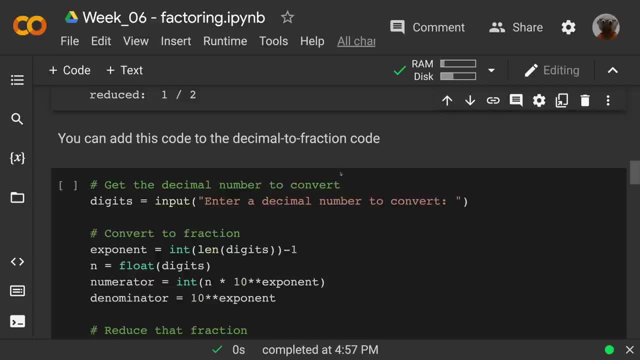 let's just do this. So we had the decimal to fraction code and you know this one. we had an input rather than just have the number here. I have this input. I asked the user to enter a decimal number to convert And remember. 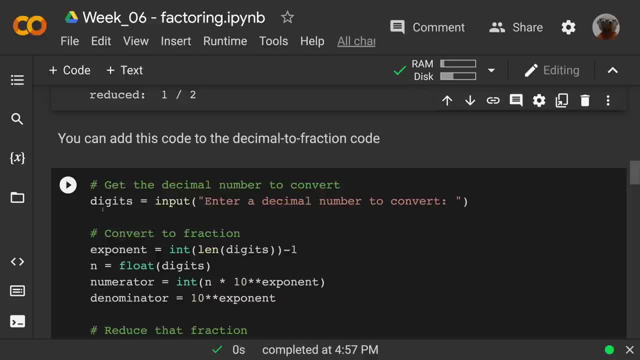 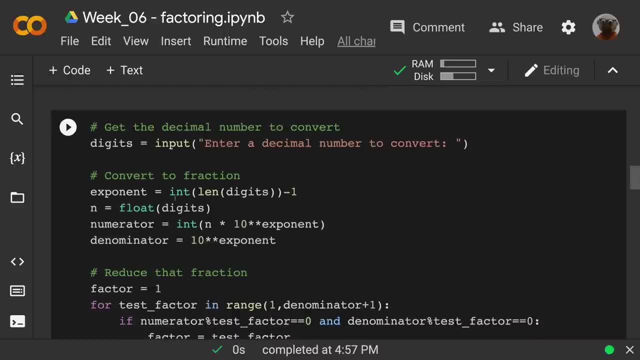 then that input gets stored as digits, but it comes in as a string And we've done this before: convert it to a fraction. So I go here. you know the length of that input. you know how many digits minus. 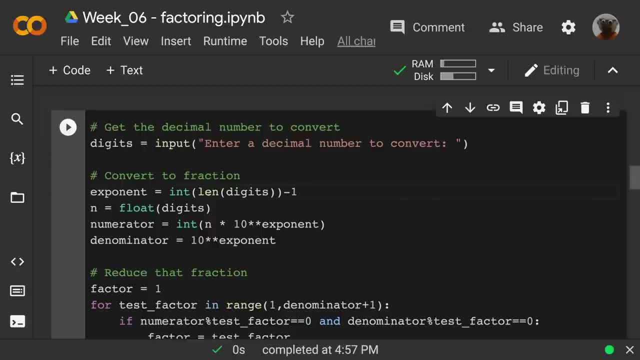 1.. Well, convert it to an integer, because I want to have minus 1, because that will come in as a string and that will include the decimal place. So there we go. Then that becomes my exponent, and then I'll still. 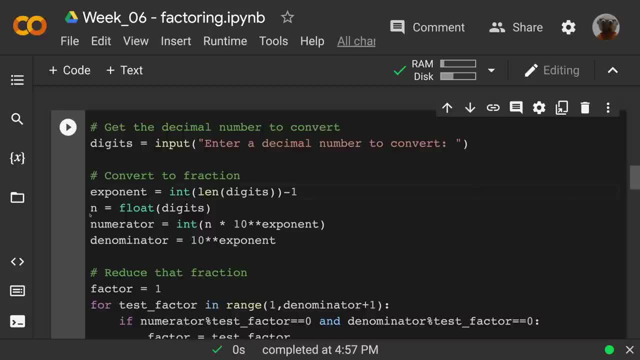 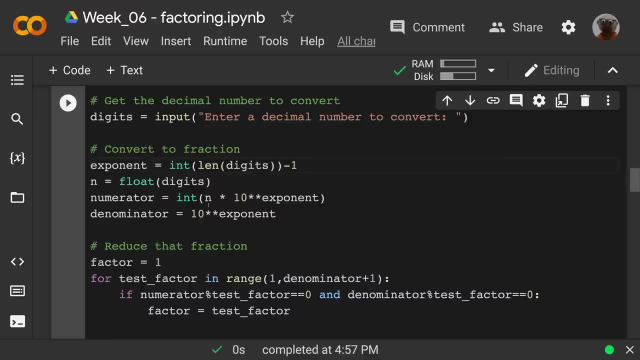 also cast that as a float number, which is n, and then as a fraction. my numerator is going to be the. my numerator here will be n times 10 to that exponent. So what that's doing is taking that value and moving the decimal place. 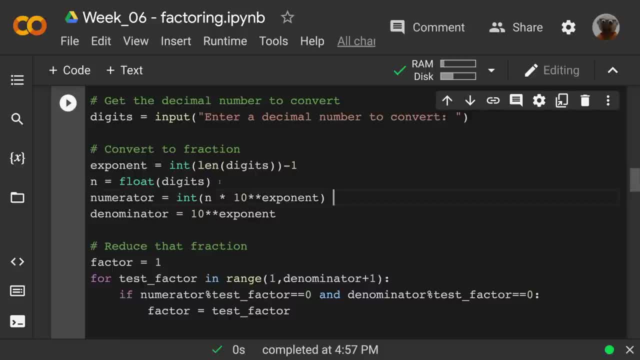 So there we go. So n has all those digits, including the decimal place. then this line for the numerator moves the decimal place and then the denominator is 10 to that exponent. So now I have an integer for the numerator. 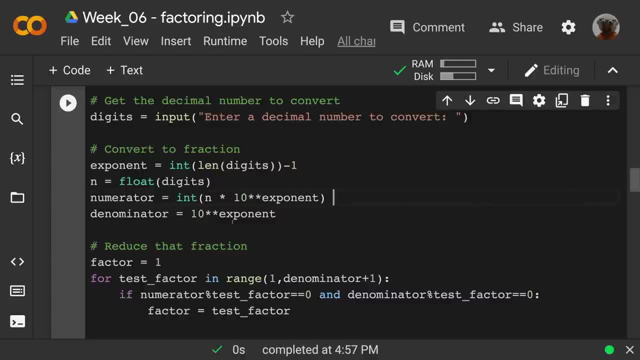 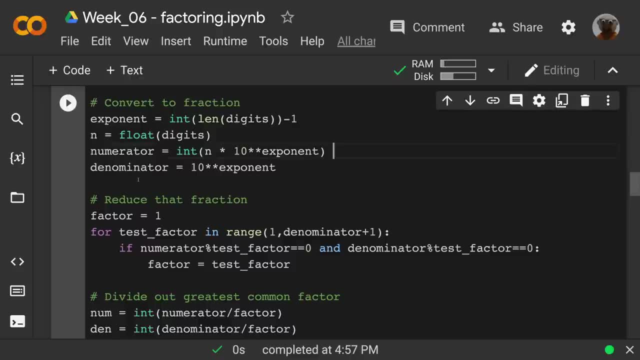 this will end up being an integer for the denominator, and now what we're going to do is just like we were doing earlier: I want to reduce that fraction. So same thing. factor equals 1,. everything else I already had. 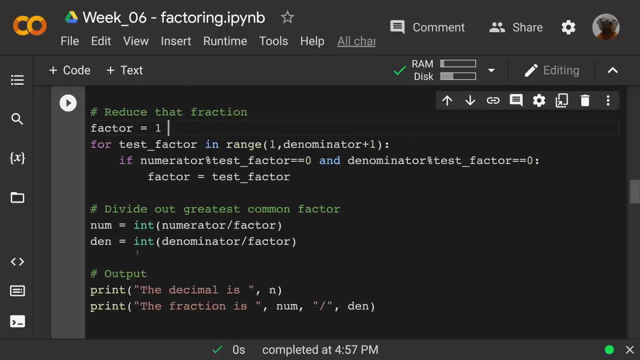 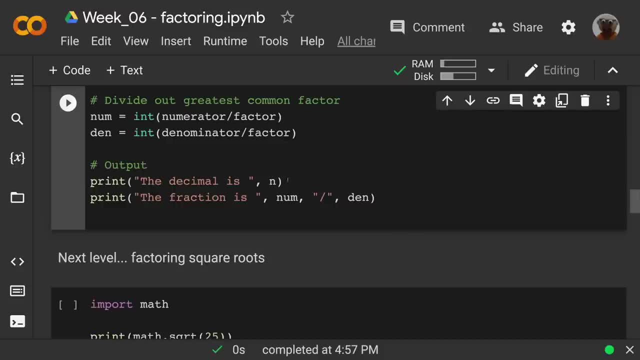 that same loop, finding the greatest factor, dividing it out. and there we go, Inputting the decimal which is the original number that the person entered, and then print the fraction. So when we run it, enter a decimal number to convert. so 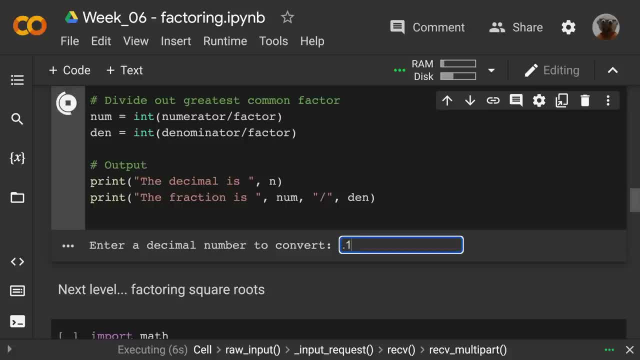 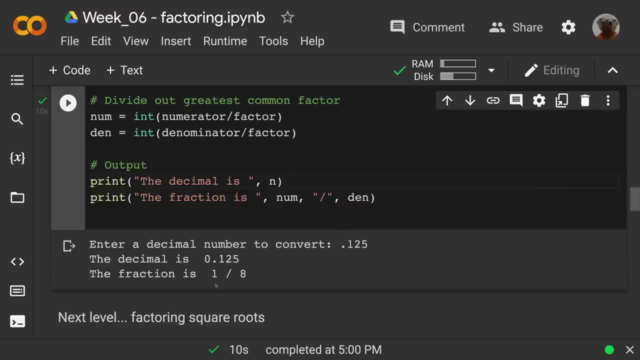 let's convert something like .125.. There we go, And it took it and it reduced it to 1 eighth, which .125 is 1 eighth, And we can run it again, just to see that if I have .02, There we go. 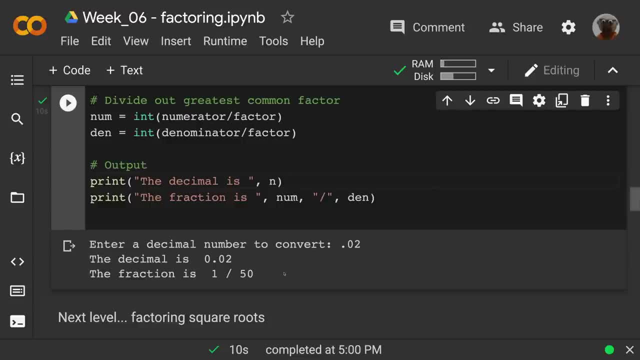 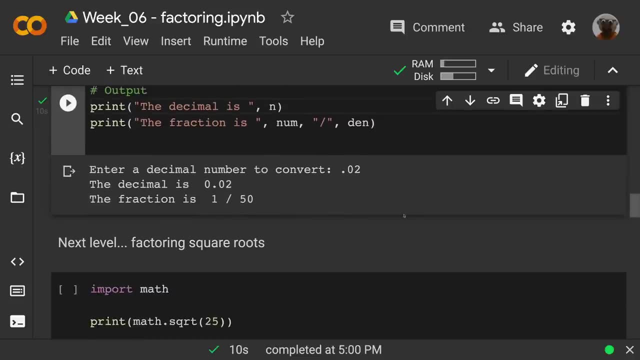 Decimal, and then that's 1 fiftieth as a fraction, So we can apply that code into other things that we've been doing. Alright, now we're going to take it to the next level: Factoring out square roots. 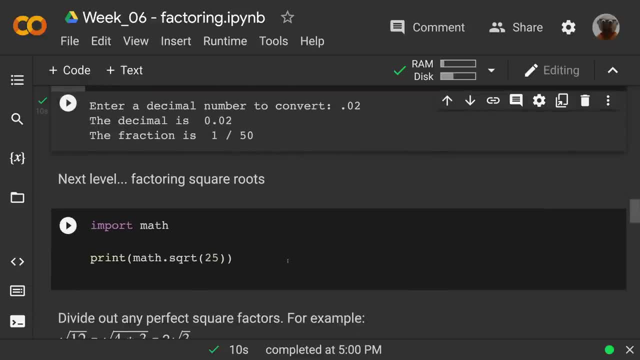 So this is all good to reduce the fractions, but remember when we square root something, now this one: if I just print mathsquare root, there we go. the square root of 25 here is 5.. Great, But what if I have something like the square root of? 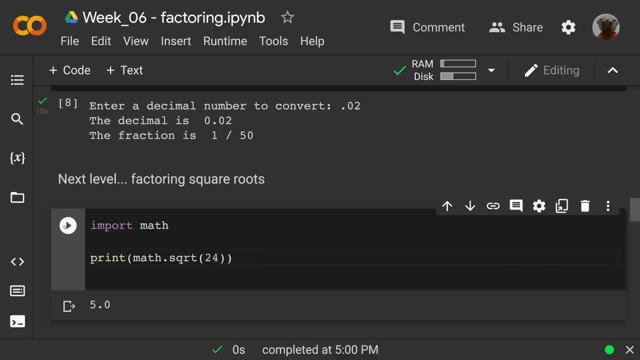 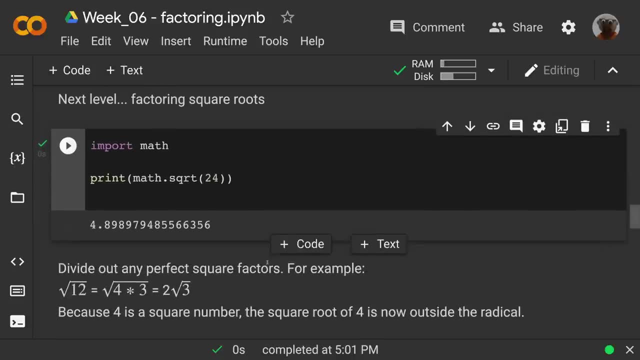 24?? Now, that doesn't work out nicely And by default it'll just give me that decimal answer. But what if I want to factor it? This is how we want to factor it. I use square root of 12 as an example. 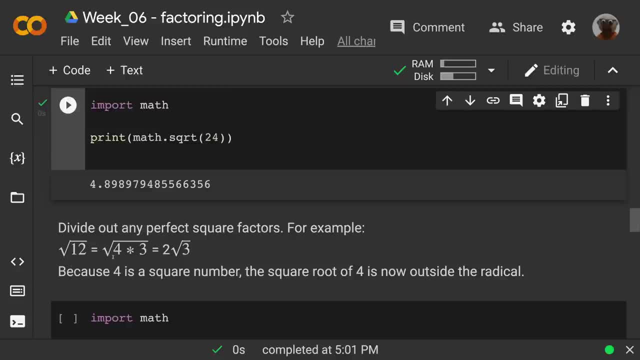 Square root of 12, because underneath the radical 12 is 4 times 3.. And then 4 is a perfect square, so the square root of 4 is 2, and that comes out, And then I have a 3 left over. Nothing else I can do with that. So that's the factored. 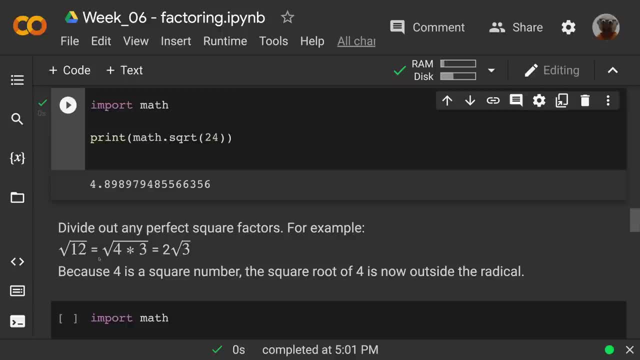 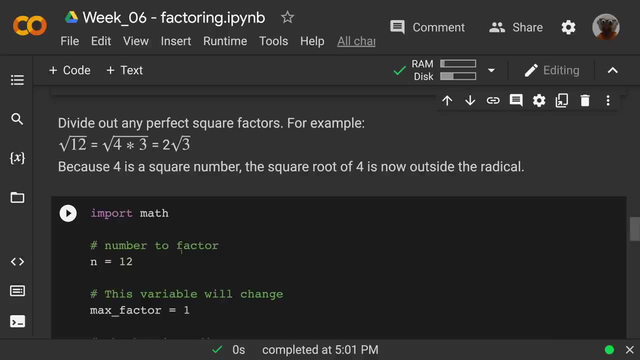 square root. We want to find our square factors and divide them out, The square root of that. There we go. So here we have number to factor. You could make it use your interface, but I just put it here: n equals 12.. 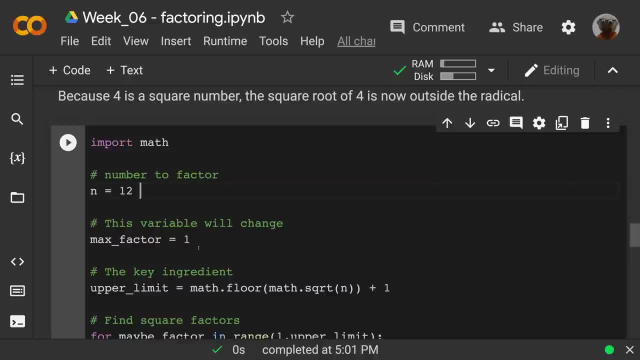 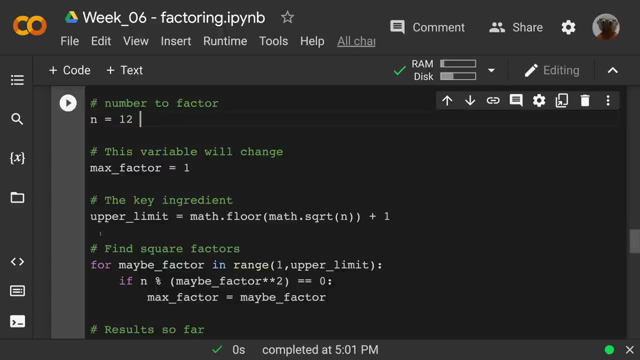 And max factor. I just made that 1.. That's the one that will change. And here's I put this as the key ingredient, because this is how we get to. you know if I have my loop, where do I start, where do I stop? 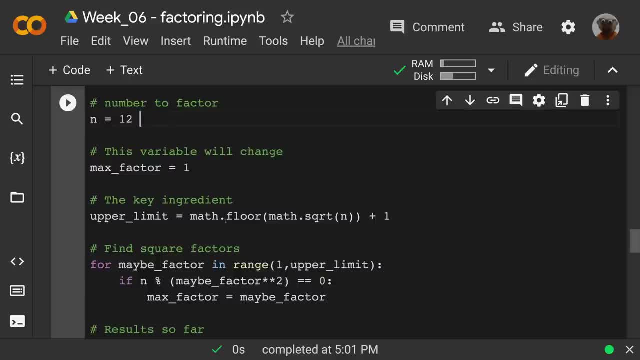 So the upper limit mathfloor of mathsqrt of n. So I'm going to take the square root of that. Then that's going to be some weird decimal number. Now I just did this mathfloor and then I added 1.. I probably could have done mathceiling also. 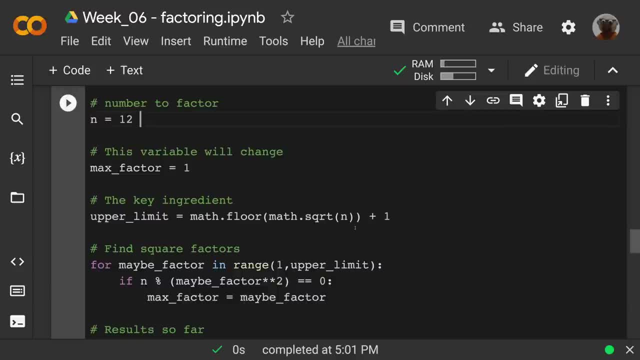 but I just did it this way. So take the square root and whatever you know mathfloor, so drop all the decimal places You know not rounded. just drop them all and then add 1.. So that's going to be the upper limit. And now we want: 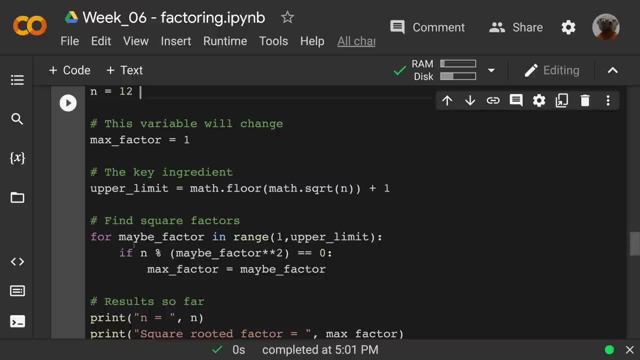 to go here. So for maybe factor in range, again, starting at 1, 0 would give an error, The upper limit if n modulus maybe factor squared. So you see, I'm running through those factors and you know each of these is the square root. 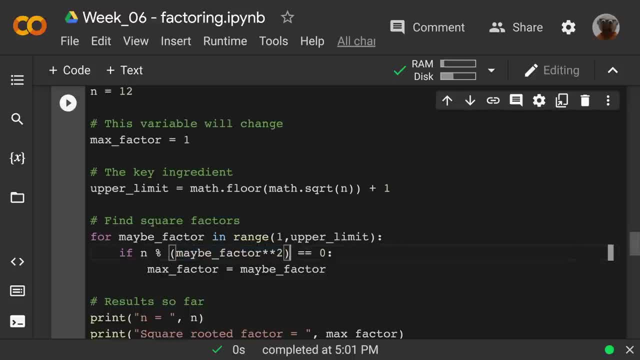 factor. So if I square n divided by that factor squared, if that's 0, then now that maybe factor is now my max factor. So we go through and we're going to cycle through all these, you know, divide it out. does this work? And once I get some, 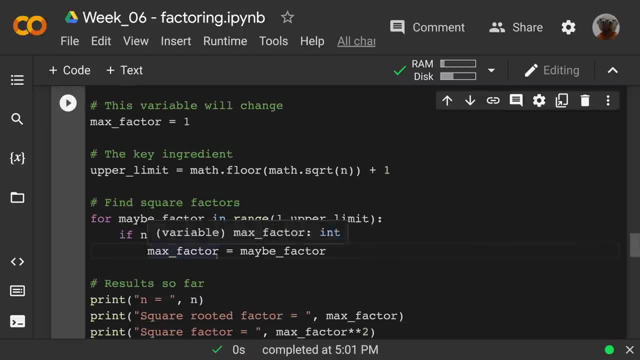 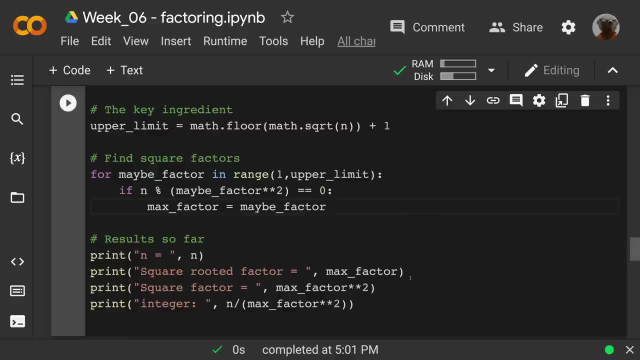 factor. that's what's going to be on the outside. So then I have the results, my original number, square rooted factor, square factor. and there's a reason why I'm printing all of these out here like this: because we're going to build upon this and make it look nice in the next step. 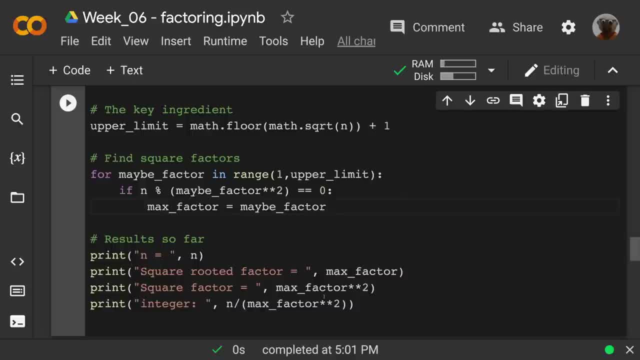 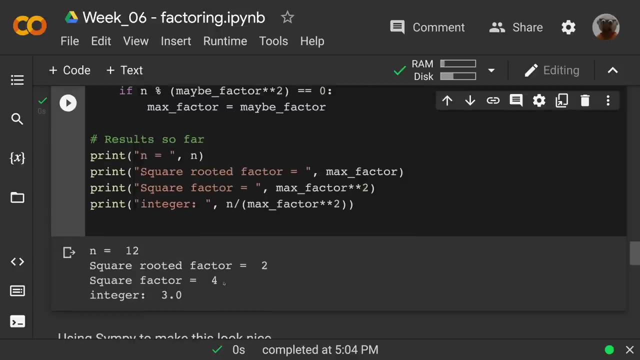 But to show that square rooted factor, square factor, max factor squared, and then the integer that's left over. So for 12, since we had that example earlier, we see that n is 12, and the square rooted factor 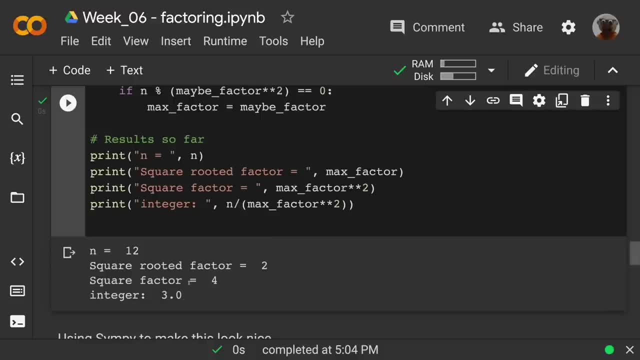 is 2,, square factor is 4, and the integer is 3.. Even though I called it integer, that was just text. it actually comes out as a float. So what we have is that this gets to that factor 2 on the outside. 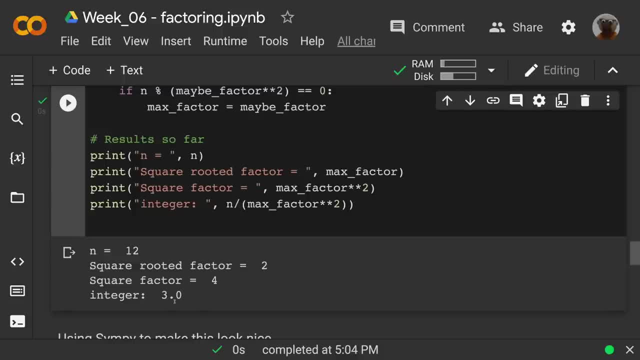 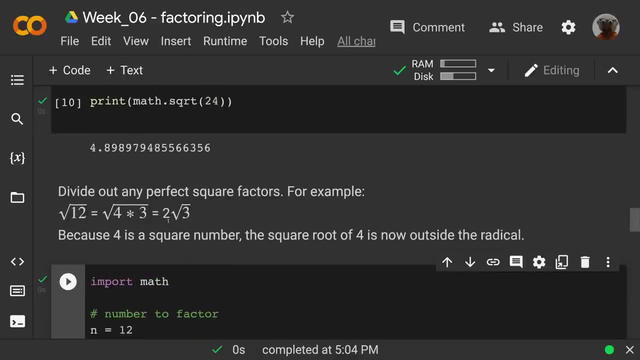 you know, 4 was a part of our in-between step, and then 3, and that square rooted factor, and then the integer that matches up with 2 coming out. that's that square rooted factor, that's the greatest one, and then 3 is the integer still in there. 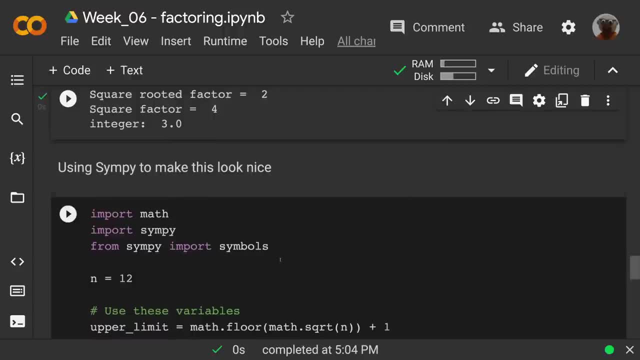 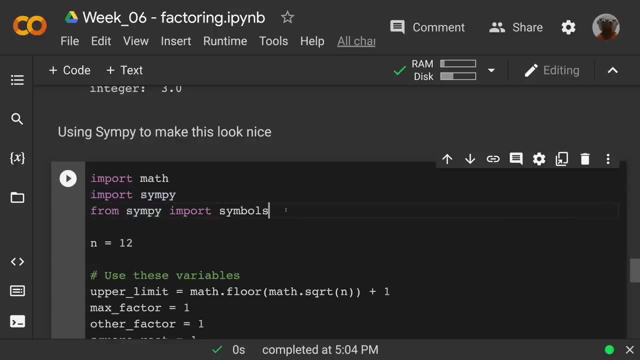 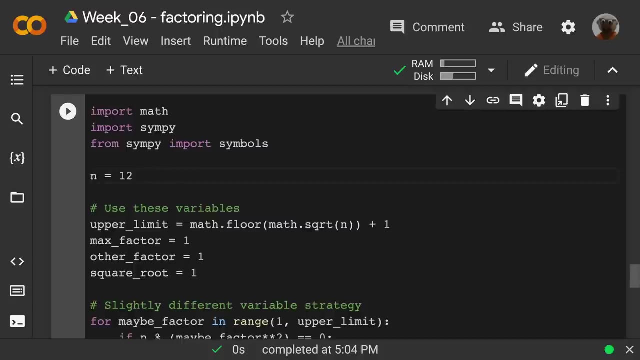 So, like I said, we're going to use SymPy to make this look nice: import math, import SymPy and from SymPy, import symbols. So now I have this, there we go, and same variables I had before upper. 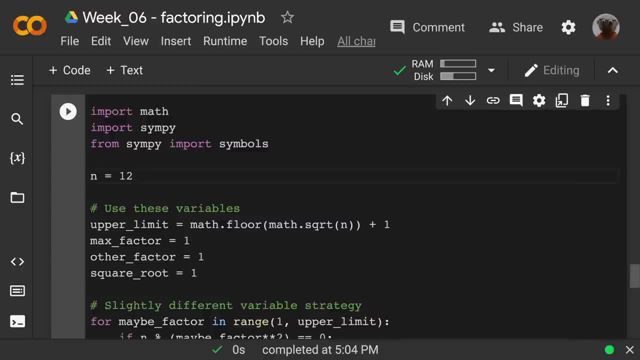 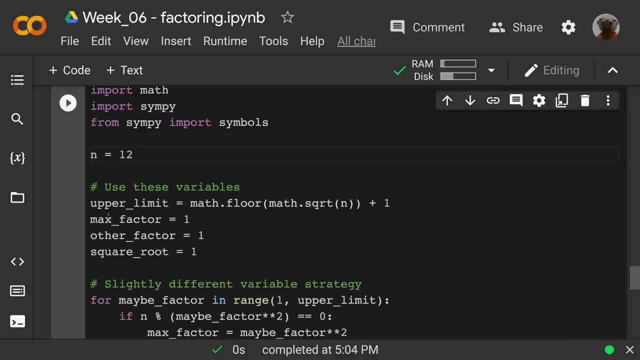 limit. there we go and it's square rooted. but then, you know, find one more to see where the maximum is going to be, Like the greatest square factor I could possibly have. So then I have all these other factor and then square. 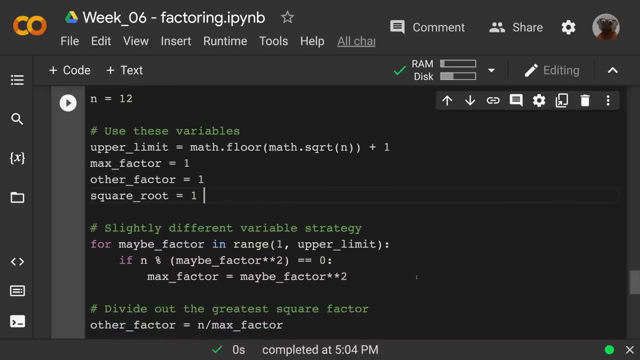 they're all starting out as 1, and I'm going to overwrite these So slightly different variable strategy. so if maybe factor in the range, if n modules maybe factor squared, then we have the max factor. is maybe factor squared, Alright, And then 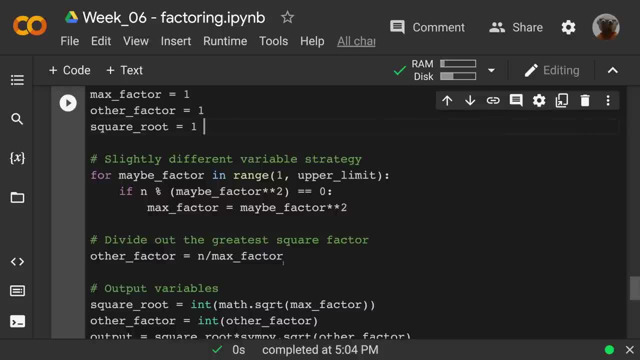 the other factor is n divided by max factor. So we see here: then this becomes the factor that I divide out, because I'm squaring it here. And then I have the other factor underneath: the radical is that original number divided by. 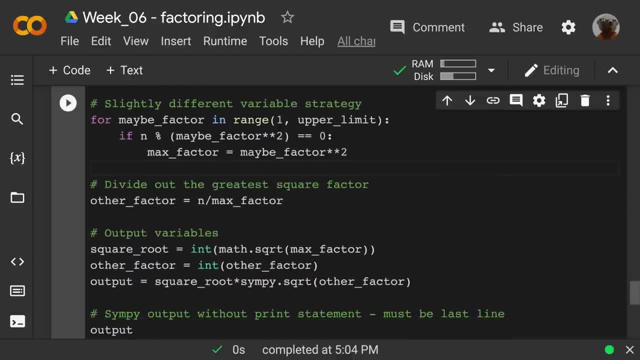 max factor, So then the output variables, and to make this look nice, we cast them all as integers. So the square root of max factor- because that's what I want- the square root of it, cast it as an integer and then. 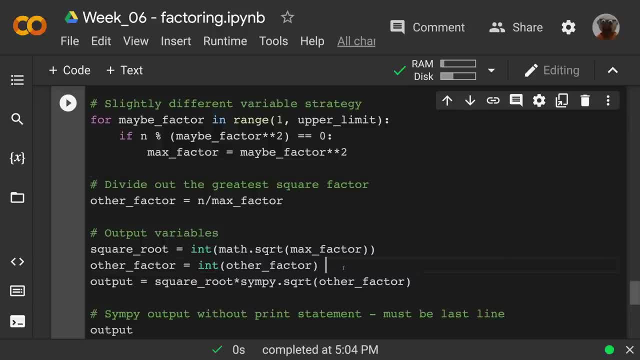 that's the square root, that's my variable square root. Other factor: cast it as an integer. There we go It. I mean it essentially will be, but we need to cast it as an integer here. other factor: 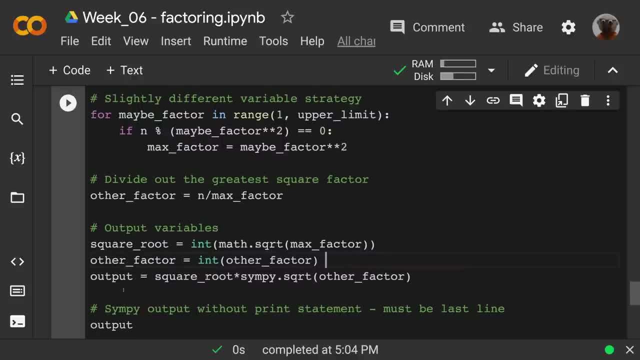 And then the output. this is its own variable output and we see it's square root times: sympy dot square sqrt. other factor. That's what that output looks like in sympy and this presentation. here we don't need a print statement. 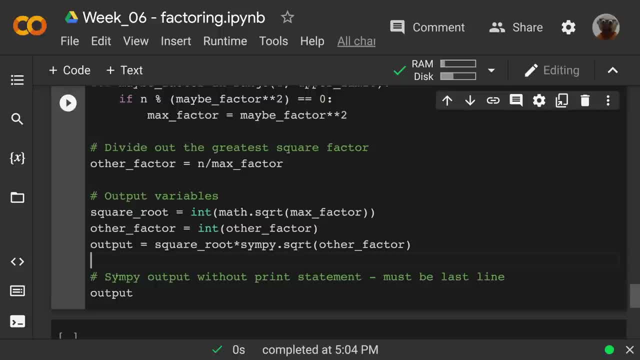 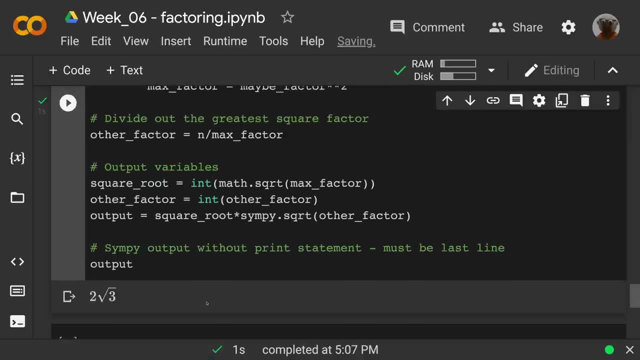 In fact that might not make it look as nice, But this sympy output. so I store all that as the variable and then, when I output it here, there we go. It factored out as 2 root, 3.. And 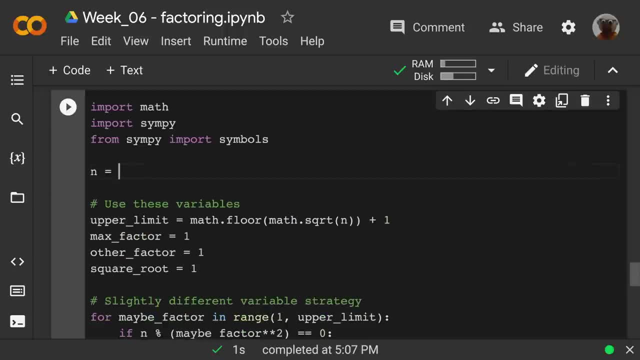 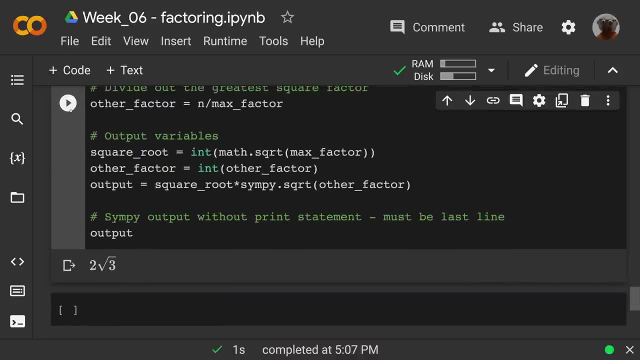 if I put it back to my other 24 that we were talking about before. we know that that doesn't work out, and so it factors that to 2 root 6, because it's 6 times 4, and then the square root of 4 is 2.. And that's what we're doing. The types of things. 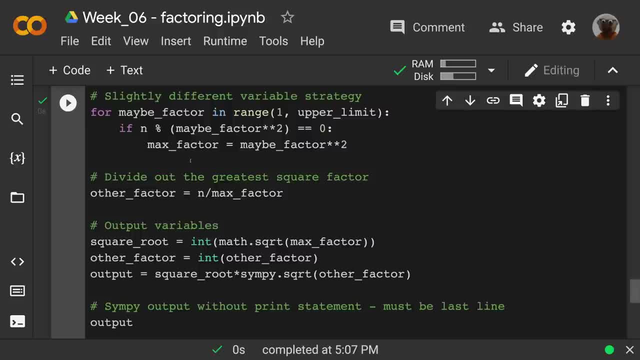 that we would be thinking through. we just want to translate that into code. You know, I'm thinking through all the factors of that number and which ones are square, perfect squares, So 24,. I want to find all these factors that are. 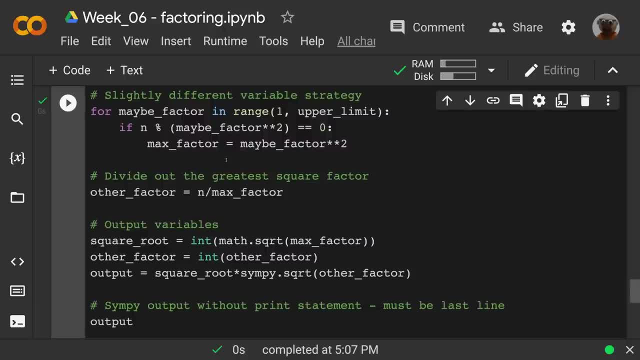 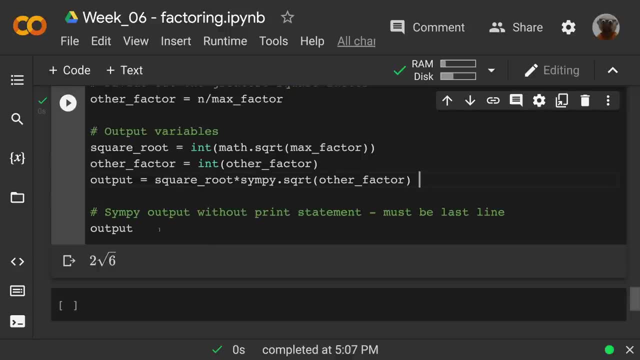 perfect square, and I find that it's 4, and then the square root comes out, And then the sympy makes it nice. So we can do this to factor square roots. and there we go. So we have this. we can divide out common factors, we can reduce fractions. 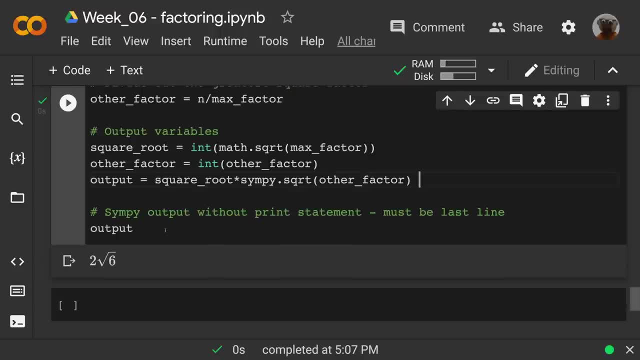 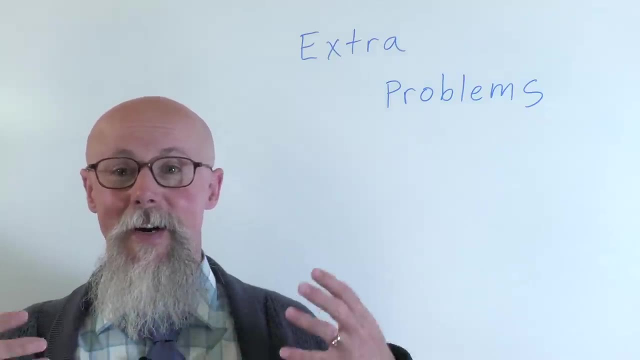 we can factor square roots, and these are a lot of the things that we often do by hand in math, and now you have the code that you can do this. Now that we've worked through the core skills in this unit, let's look through some extra problems and 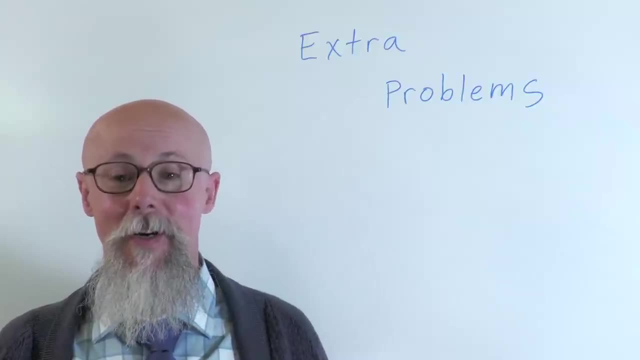 I'm going to work through extra problems using the Colab notebook so you can see how you can apply these resources that you're building and use these to solve problems that might come up in a textbook or in day-to-day life. So we're going to go through some more. 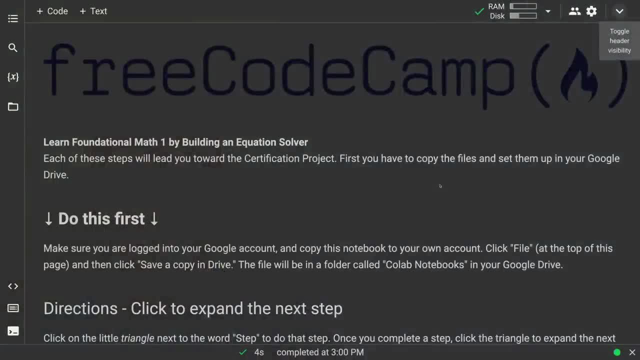 extra problems here. So we're going to do a walk-through of the first certification in foundational math Now, each of these notebooks. there's five of them. we'll do three of them for this course and then two of them in the next course. 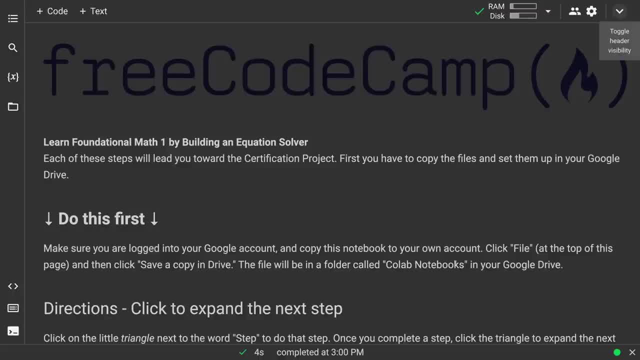 but they were all. I also designed them to be stand-alone. that you know the directions would be enough that you could walk through and be able to do all of this. Still, though, I'm going to give you the walk-through. 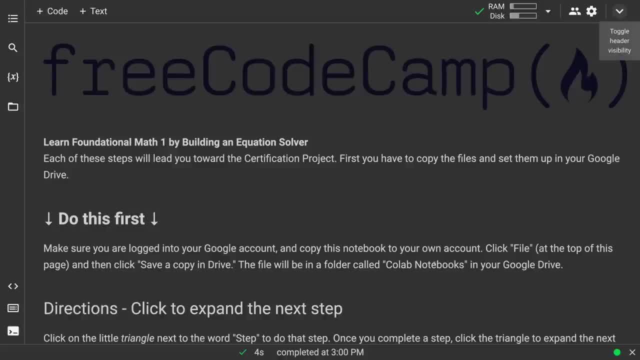 um, maybe you already did this and you want to check some things, or maybe some of it didn't, uh, turn out as you expected, or you're stuck somewhere, so you can always jump to that spot in this video and see So. 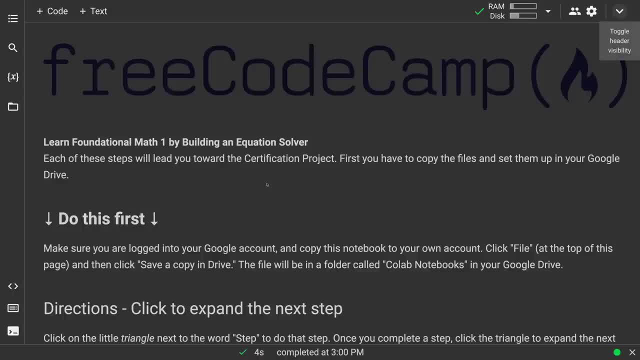 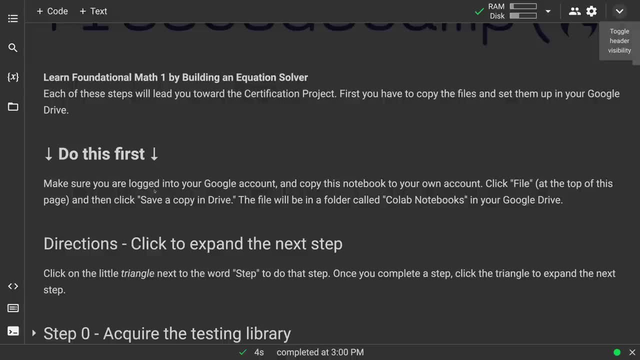 each of these steps lead you towards a certification, and you know we build upon each thing, So the first thing you're going to do is make a copy of this whole notebook. This notebook is read-only and this is what gets shared out to everybody, so 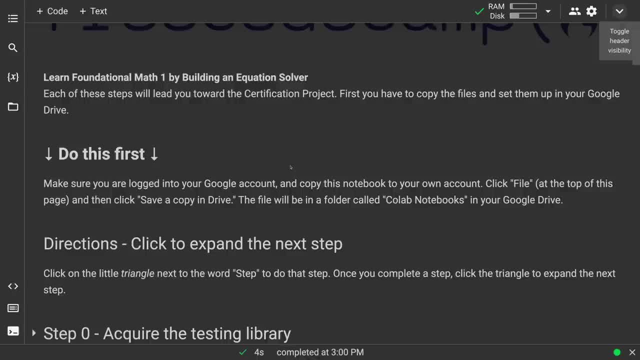 you make a copy and that copy's going to be in your Google Drive, Uh, and it will be in a folder called CoLab Notebooks by default, but if not, you can put it in whatever folder you'd want it to be. 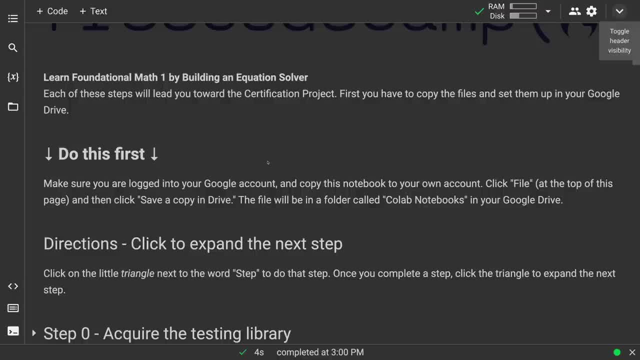 you want it to be in, and this is the ongoing theme for this course. you're building your resources, so you're going to put this stuff in your Google Drive, uh, especially if you have other CoLab notebooks or something you could. 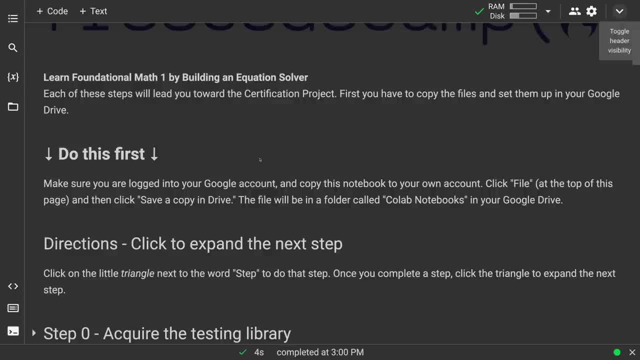 make a different folder for everything, uh, in Foundational Math 1,, you know, or Algebra with Python, if you want to call it that. So you make your own folder. you're putting all these resources in there that you'll have, so you walk through as. 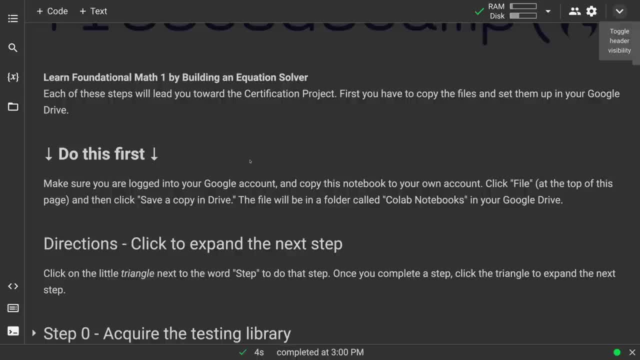 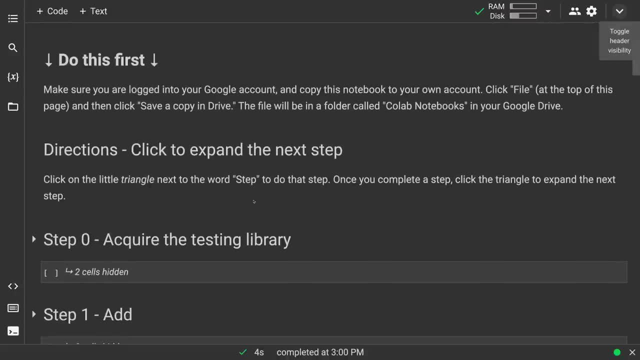 you work through these, you'll understand how to do all these things, but then you also have some code that you can reference, So you have this in your Drive. I already did this. and then each of these I have as a different section heading. 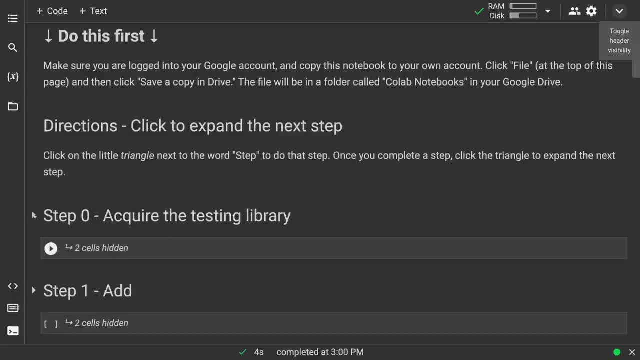 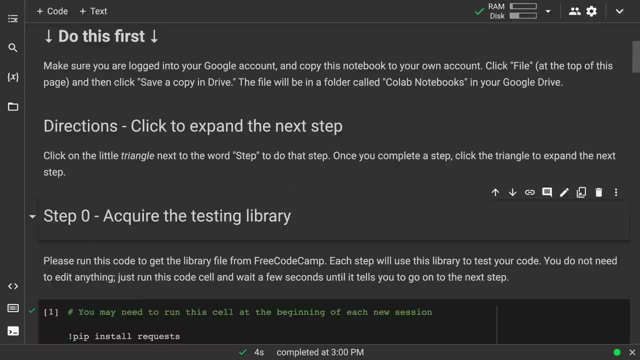 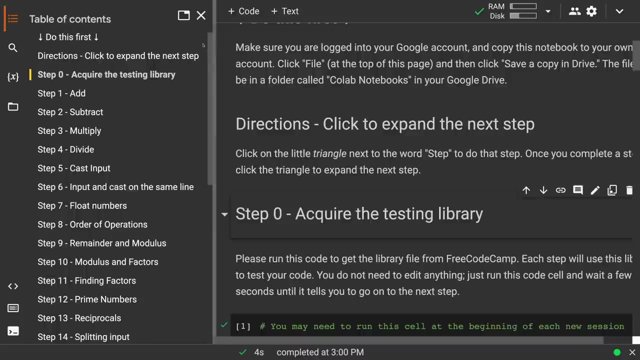 and then you can click on the triangle here to expand the next step, And with each of these being section headings, then up here you have a table of contents that you can go through. so later on, when you build yours, you can jump to whatever part. 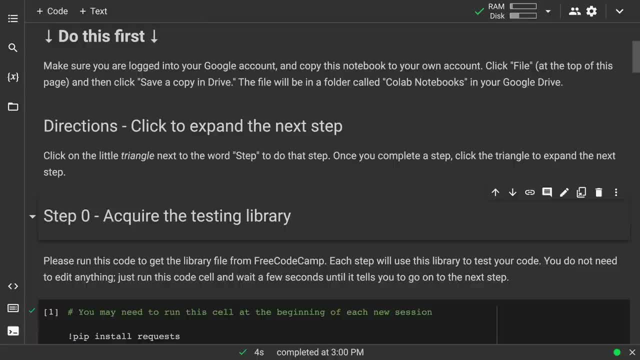 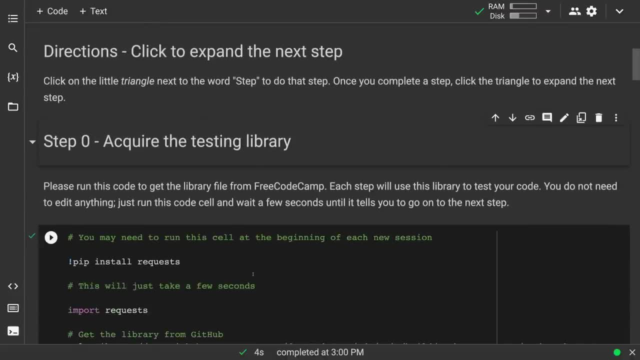 you want. You know you can add the table of contents by just making each of these a section heading. So you do need to acquire the testing library, because this is actually self-contained: you're going to write the code and then it's going to test the code that you wrote. 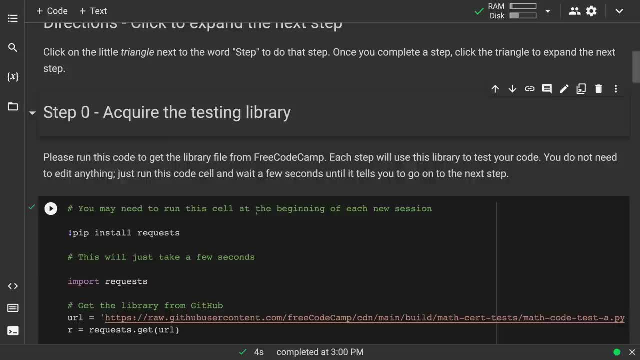 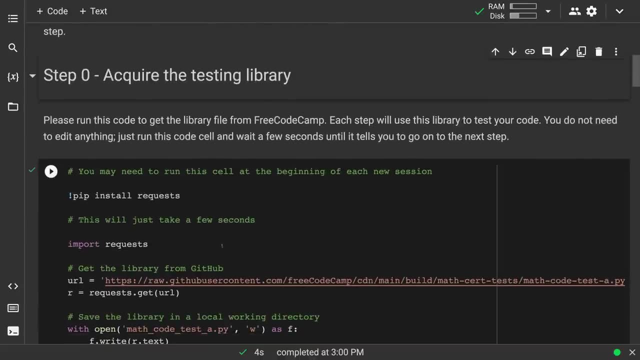 and see if it's correct or not. So this cell, you don't need to do anything to it. maybe for other things you might do in the future you might take notice of. you know how we import this other library as this raw. 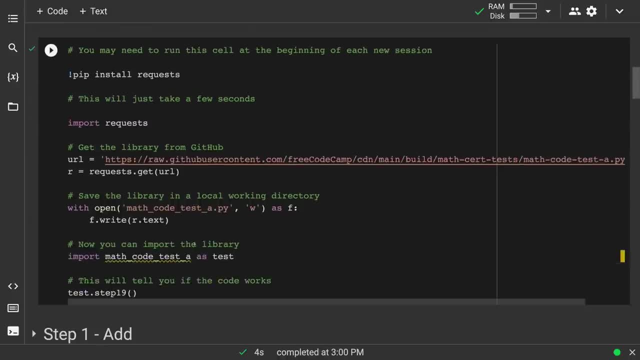 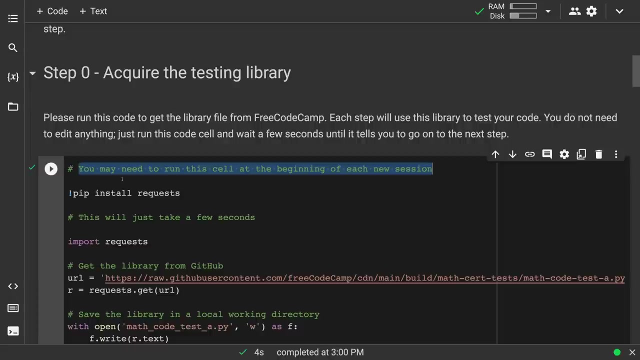 py file in GitHub and really save it as a library locally here, and then you'll be able to access it. So this I have the note here. you may need to run this at the beginning of every session. And the only reason I said may is because 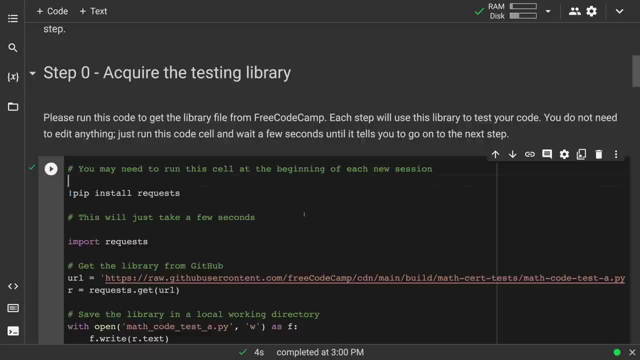 maybe if you walked away for two minutes and come back, don't count that as another session. But these Codelab notebooks, they do timeout. The runtime will timeout after 30 minutes of inactivity. and that doesn't mean no typing, that means no running any cell, Or even. if you are really active all day, it'll timeout at 12 hours. So then you, you know you might say: wait, I haven't. I've been active all day, and why did it timeout? They have that timeout too. All these are security features. 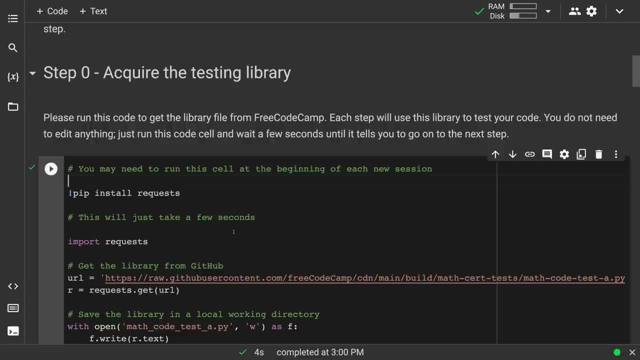 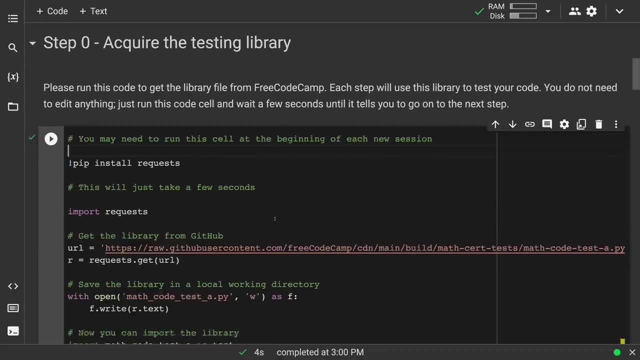 so you don't just like leave it open for, you know, indefinite amounts of time. Alright, so you're just going to get this library and you're going to run it, and we'll take a look at this. So 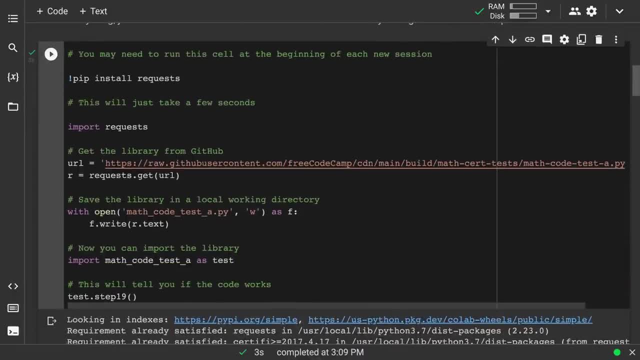 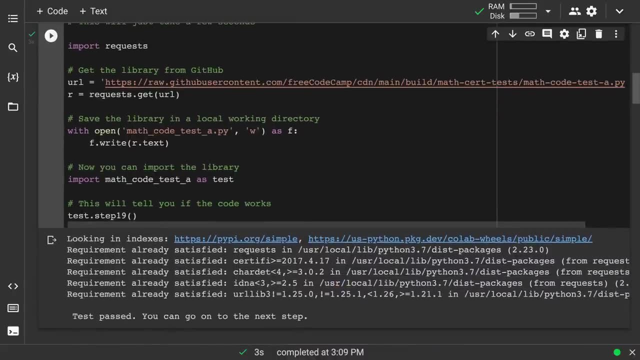 click run and, as this is going, yep, it'll save the library locally and then that's what it's going to reference. So it'll say: requirement already satisfied, Even though it said that. don't think that. oh, why did I? 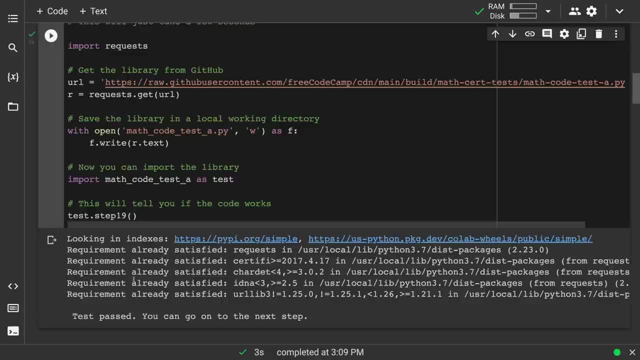 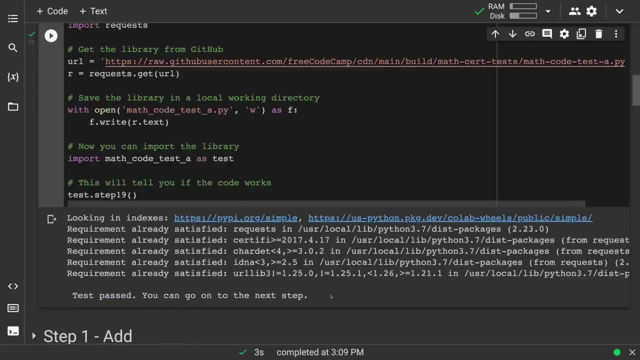 do this. It was already okay. That's just what it prints out And then, when you see this test pass, go on to the next step. then you know you're good. So it imports this and you know, now we have this library available. 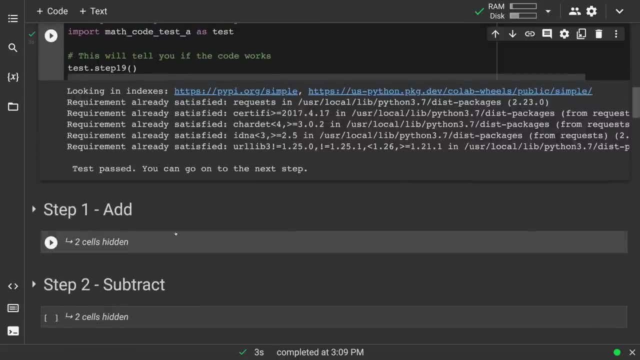 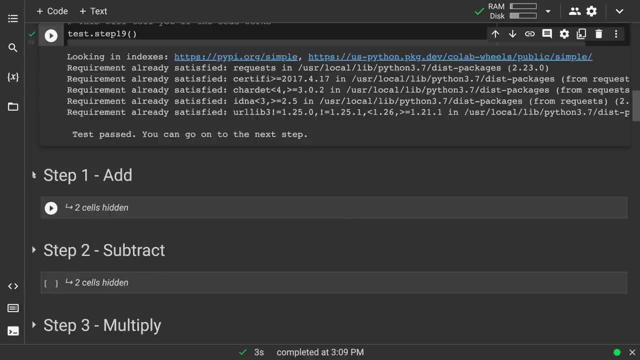 and each step will use that to test it. So these first four: yes, I do have add, subtract, multiply and divide. I know you know how to do these. You probably even know how to do them in Python, but it kind of walks. 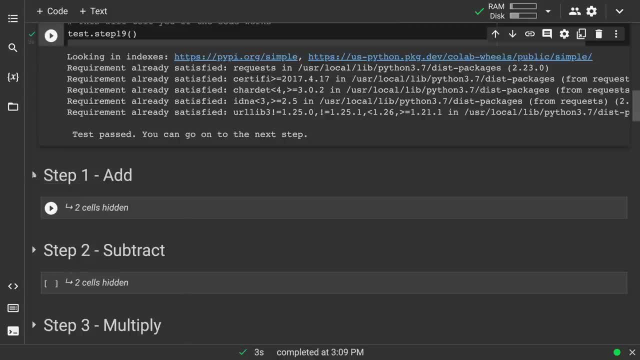 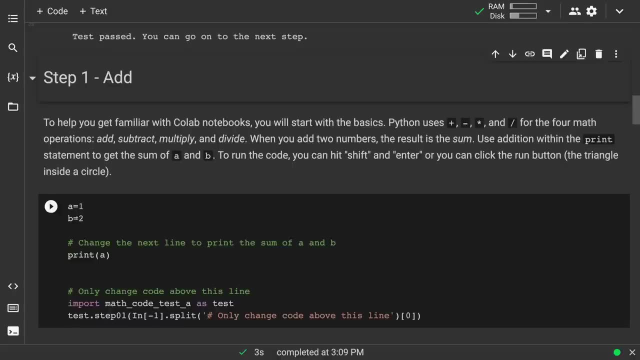 you through just gradually getting familiar with the notebook. You might be already familiar with it, but you know we'll take a look. So we go through just you know two variables and then you're going to have one thing here. 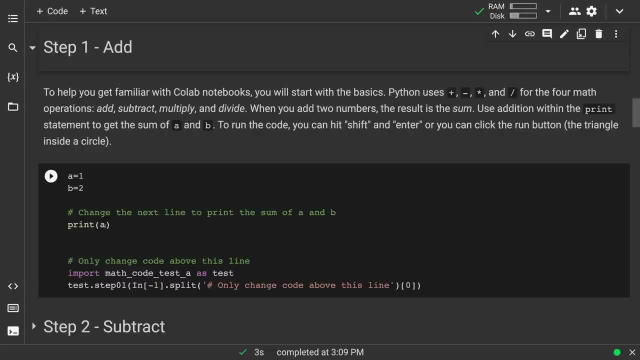 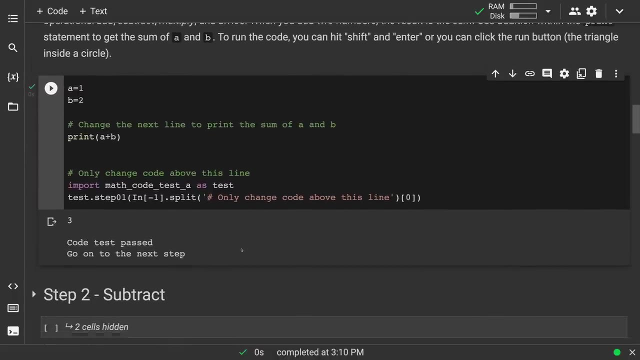 with the comment: change the next line. Now, this was just add, so there we go. I'm just going to do a plus b and I'm going to click run and you see two plus one is three, and then it said: code test passed, Go on to the next step. So we go to. 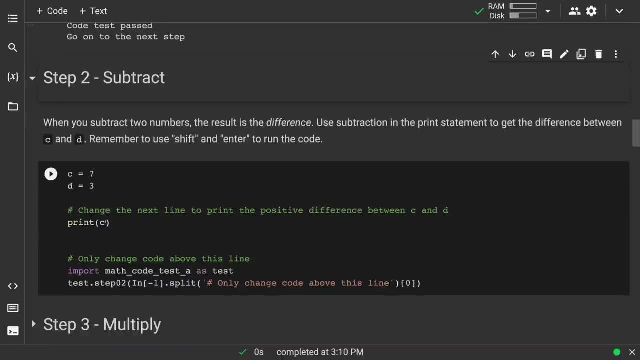 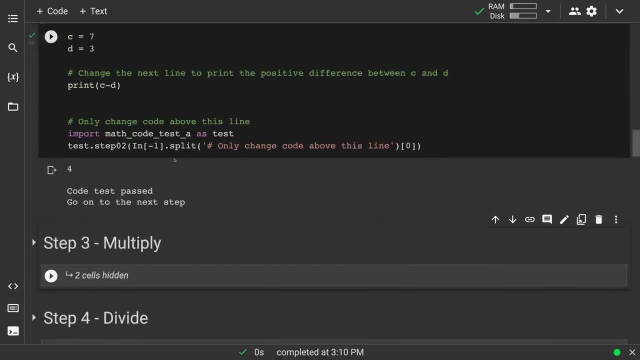 the next one subtract seven minus three, so I'm going to do c minus d and I can hit run, or I can hit shift enter, which I'll do. that time Code test passed. So this is just getting you familiar. and then each of these imports: 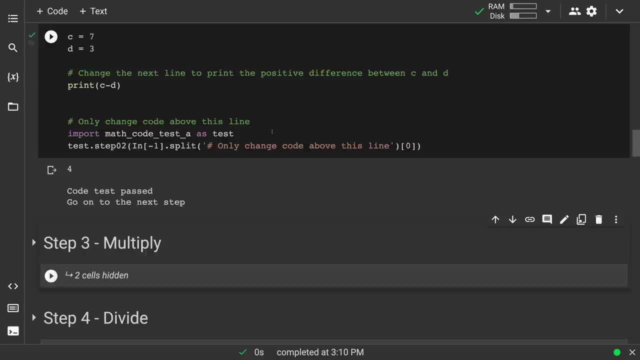 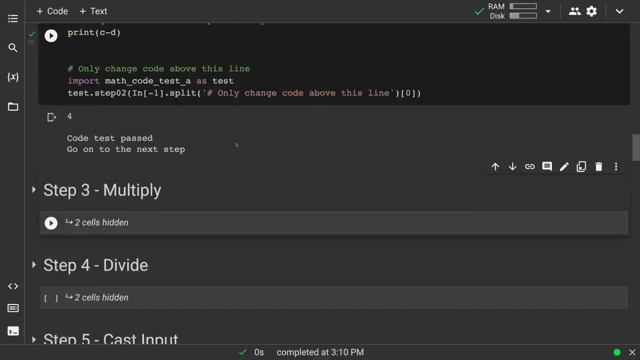 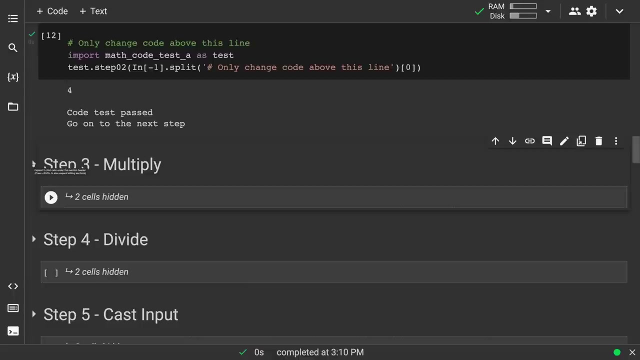 the test. So you run that first cell and then you have the test and that's what's going to check your code and tell you One of these steps. in a little bit I'll do one that gets it wrong and you'll see what it'll tell you. So 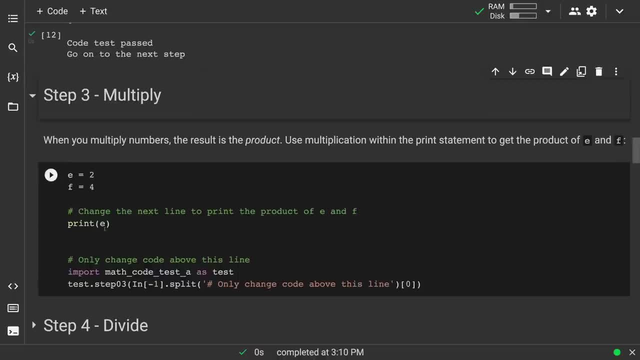 here we go. So we'll expand, multiply and again remember: multiply. in Python, like a lot of things, is the asterisk same key, or most keyboards same key as the eight. so just hit shift and it's above the eight. There we go. e times f. 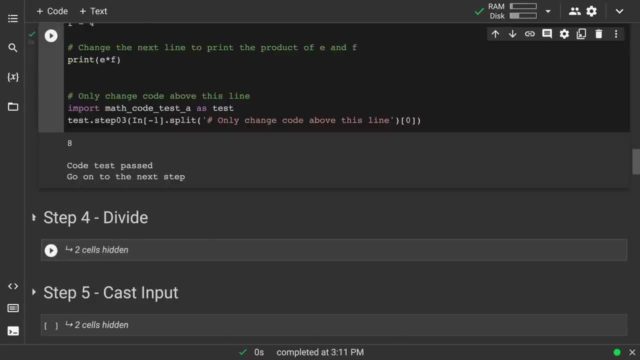 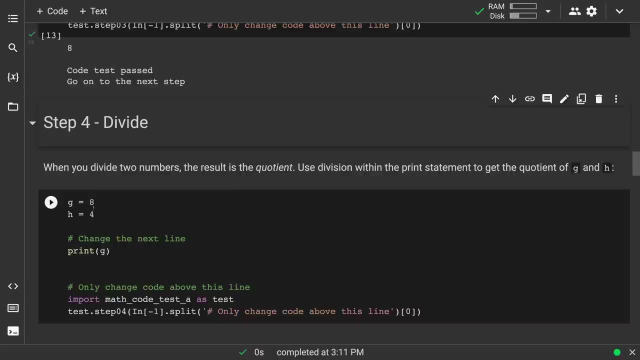 All good, Code test passed. and then we divide. Now, when we divide here g and h, now they happen to be integers and this happens to work out. but if I had them as numbers, that didn't work out if they were. 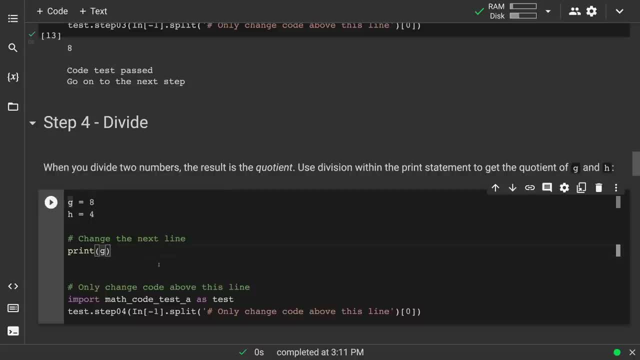 definitely defined as integers, then I would have to do something else, because if I divide the answer, and if I divide and it won't work out, the answer will be a float. But Python gets pretty flexible with this, you know, I just define. 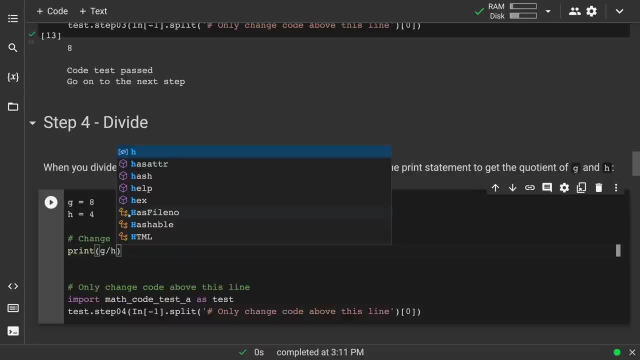 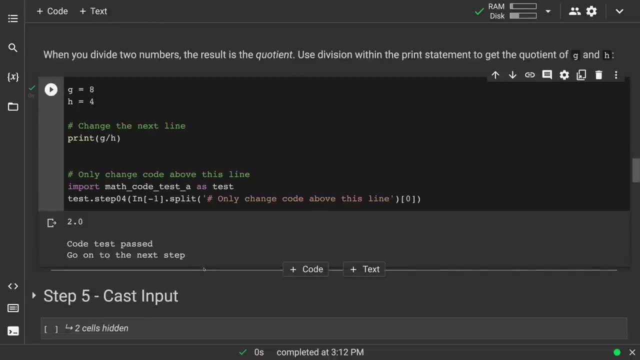 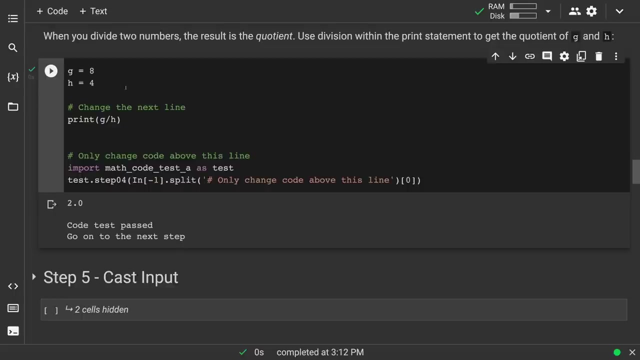 g equals, h equals, and when I divide, it's not going to give me a hard time about whether they're integers or not, It's just going to divide and there we go. So you can and a lot of things that you might work through here. if this is your notebook, you might just have things where 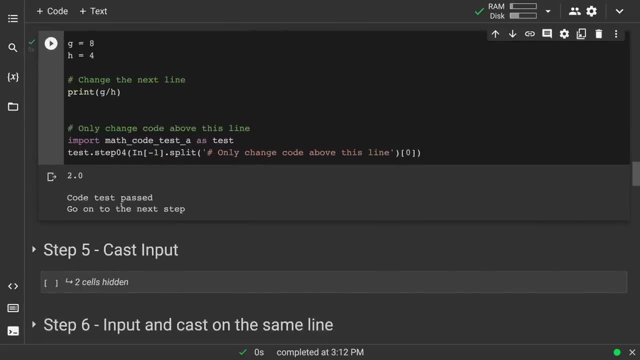 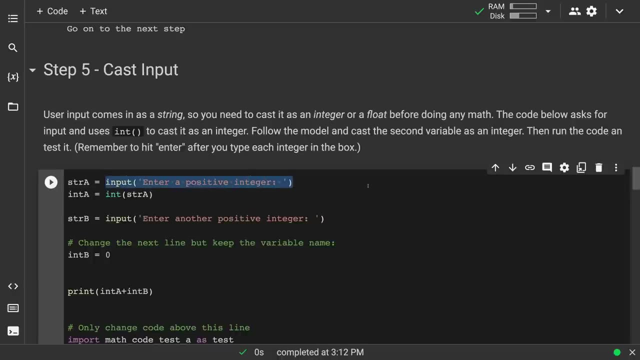 you define your input or your variables right there in the code, but you could also actually just prompt for input, And so in that case you don't have to change the code, because when you run it it will prompt for input, and then that could be the different numbers that you want. 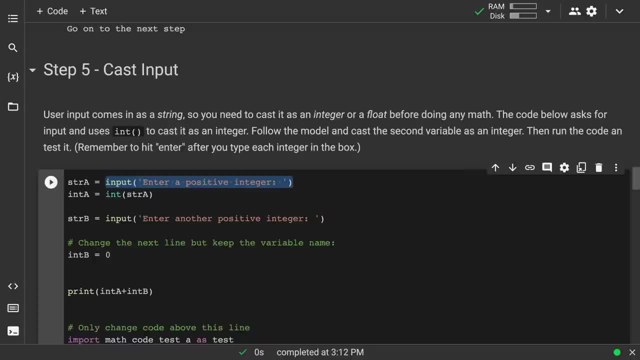 That way you don't have to worry about changing the code. So in this case, enter a positive integer. it actually could for what we're doing here. it could be negative, but I just put that there and then we just cast it, because the input always comes in as. 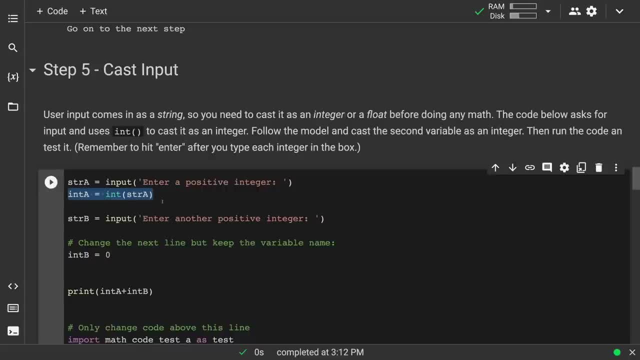 a string, and then I need to cast it, in this case as an integer, to do some math to it. Alright, so I need to do an integer or a float, and then the only thing you need to do here is following that model I have. 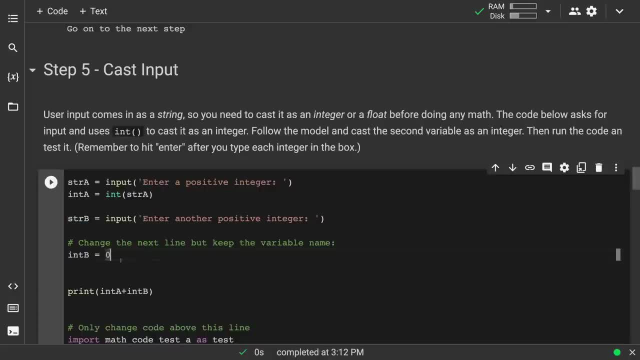 string b and a lot of these have some code, something there that won't break the code, but you do need to change it. It's not just zero, it's going to be this And you absolutely could just copy this And paste it. 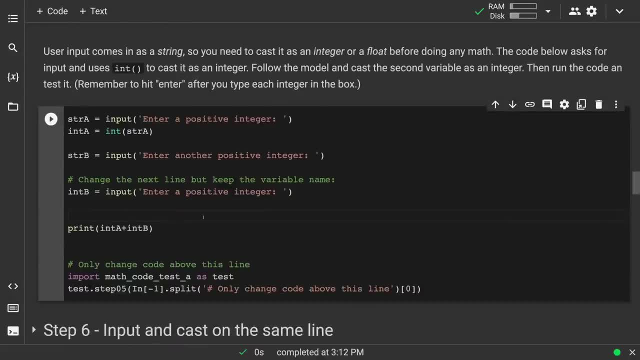 There we go. Now. what if I just change this? Now, that's really all you need to do. but what if I just said: oh, just for me, I feel like you entered one. I want to say: enter another. 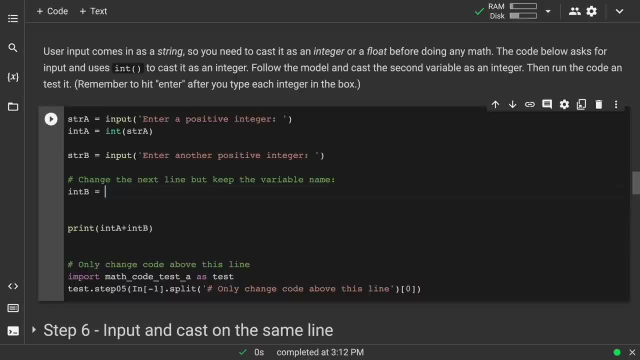 Oh, and I copied the wrong one. I want to cast it as a string, I want to cast it as an integer. So string b: Okay. so if I have that Now, I don't need to tinker with this at all. so I might not, but if I wanted to, 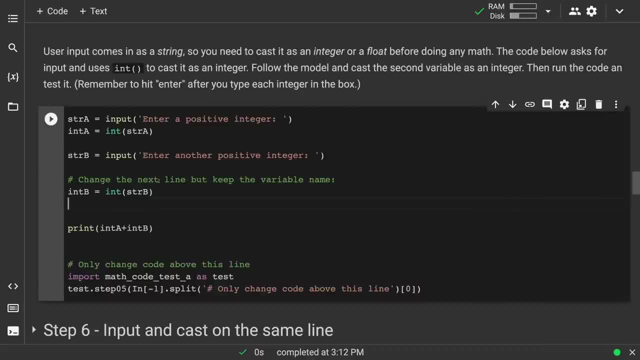 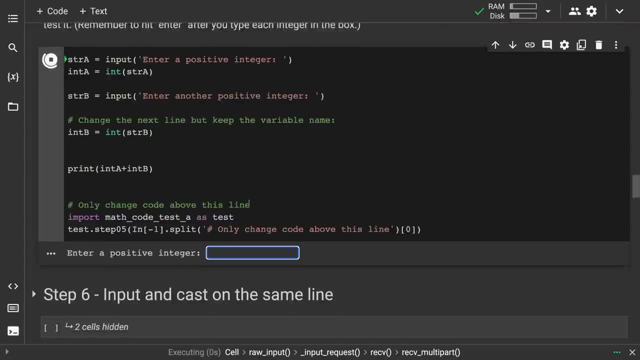 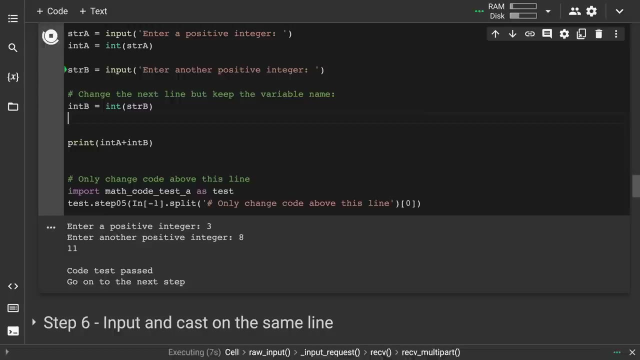 change this to another or something like that that you know we'll see. Alright, so enter a positive integer, another one. eight, there we go. So what I was saying is if I wanted to change some little things that might not be central. 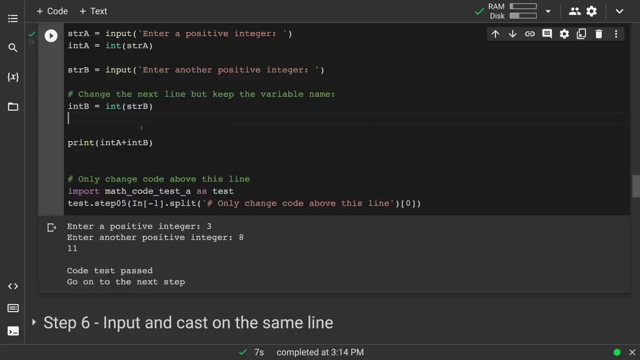 even if it gave an error, it shouldn't stop you, Alright, but this case, yeah, casting it as an integer and adding it, we're fine. If I cast each as an integer and then I went to divide, it would give me an error. 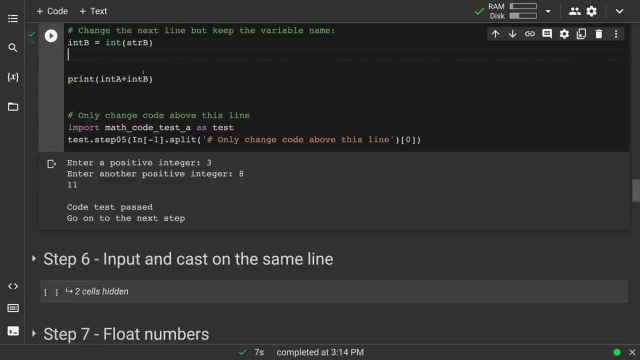 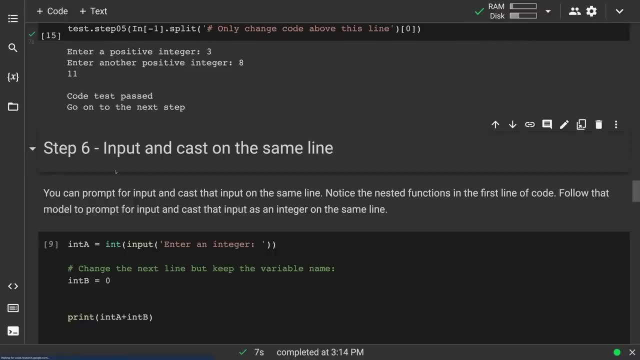 But I didn't want to worry about that, for right now we're defining them as integers. we're just adding: we'll cross that bridge when we get to it And we can get input and cast it on the same line, So notice. 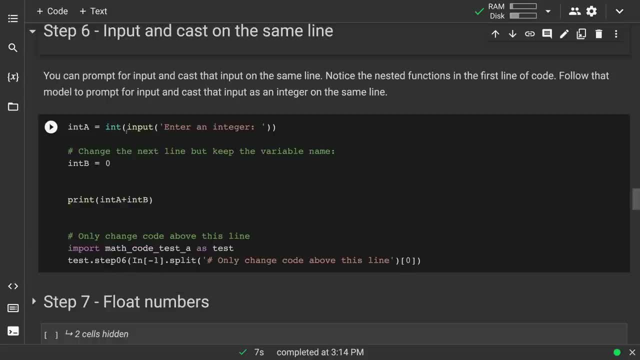 just open parentheses. there we go, and I'm going to do the same thing here. I'm going to copy this whole line, because that's really what I want to do. Alright, now here's one where I really don't need to do anything else. 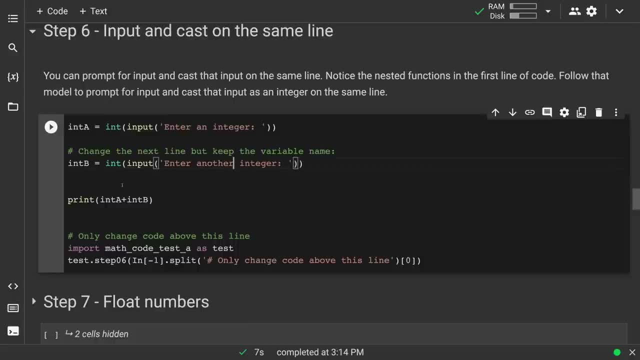 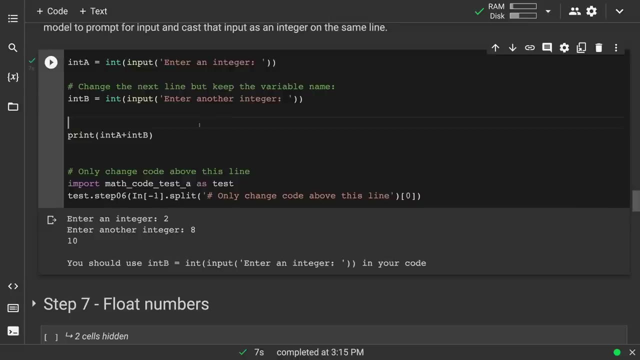 but supposing I just change that to another Now, just the way I have it. See, it actually just tested a bunch of these things because that's part of the line and I really didn't need to change that word. So it'll tell me. 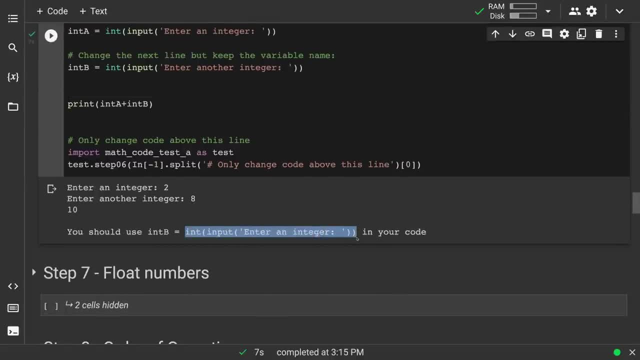 hey, your input should be this. Now, my point here is: this will not prevent you from going on to the next step. So maybe that's it. maybe there's something little in there that why did it say it was narrow? it looks correct, or something like that, and maybe 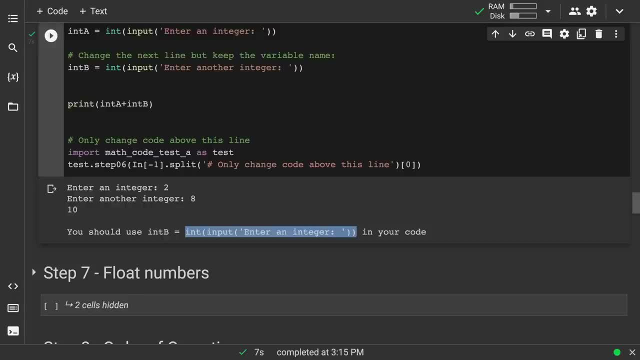 you're watching this video because that's where you were stuck. It should not prevent you from going on to the next step And in fact, that's fine. you can say, alright, I see what was different, I'm not worried about it. on to the next step. 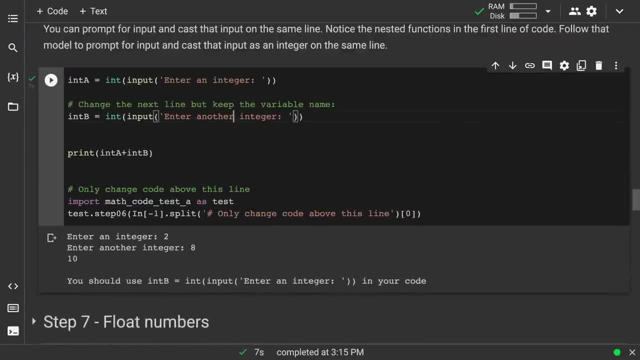 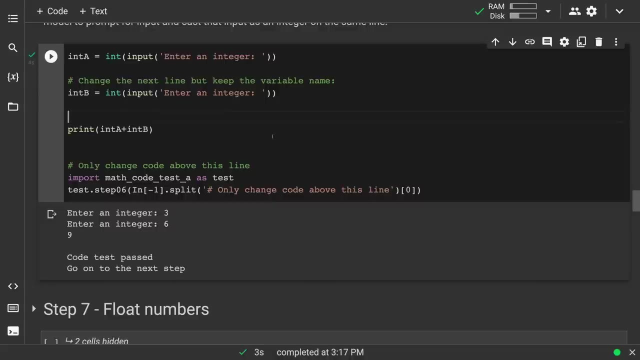 But if you wanted to, you say, oh, okay, well, maybe I should have just said this: you could always go back through and check it and then see, there we go, And then you can make your change. So the whole. 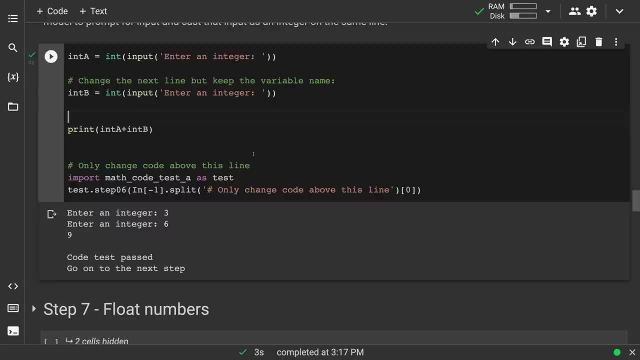 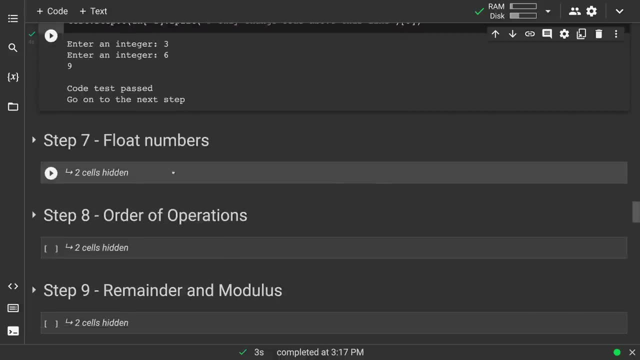 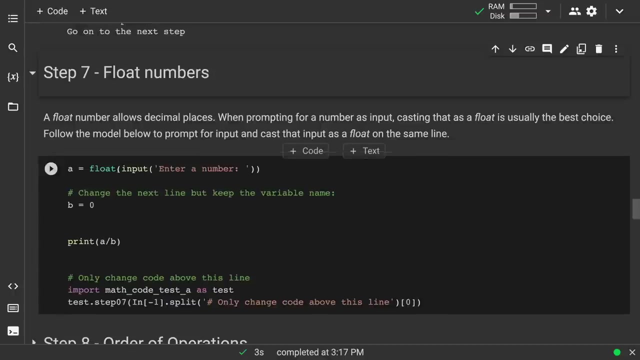 thing is that this is supposed to be just a teaching tool. check your code and then move on, but you know not to change that. It doesn't get you caught in something that you know is preventing you from moving on. Alright now. 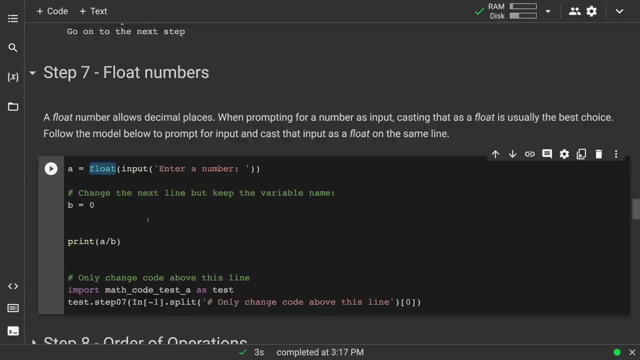 as I was mentioning about dividing, casting things as a float. So the float number allows for decimal places and most of the time I'm just going to cast things as a float anyway, Because just in case, somewhere along the way, I need the decimal places. 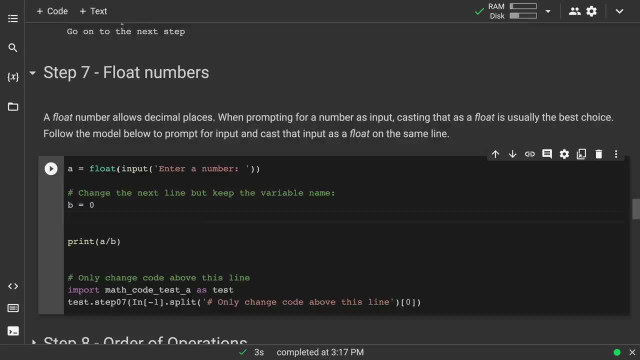 There's only a few situations where I might definitely need an integer, Certain SymPy things to display. we'll get to that soon enough- and counting but other numbers that I'm going to do math to it, I'm going to cast it as a float, Okay so. 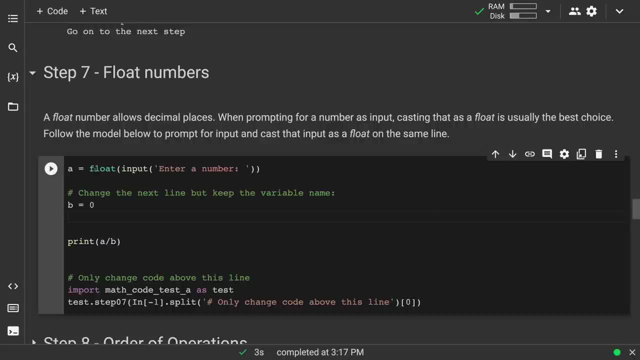 again prompt and then cast as a float. we're really just going to do the same thing And that's okay. you need you know if you copy, you need to know what line to copy and need to know exactly where to put it. 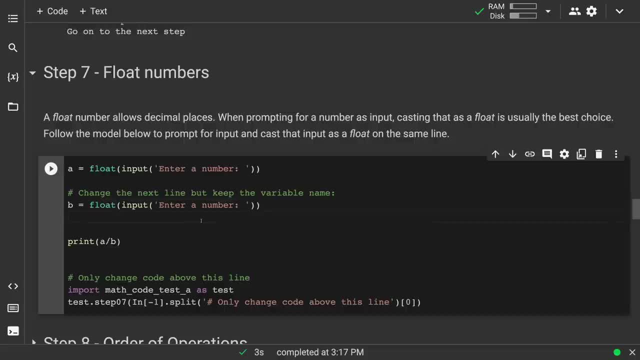 But there we go And we don't need to change this. enter a number, enter a number and see. now we will divide. so I definitely want them to be floats, because I didn't even say integer, I just said a number. 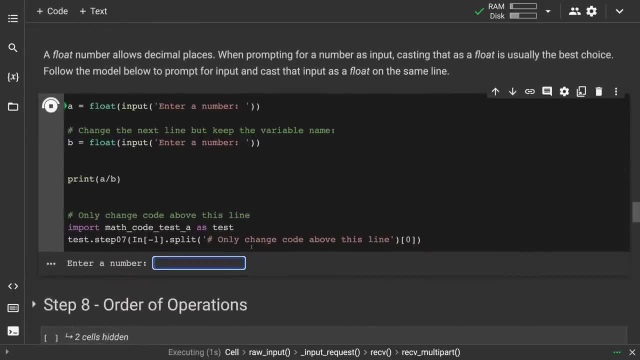 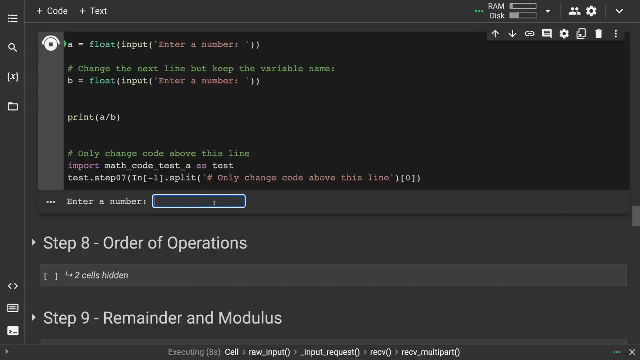 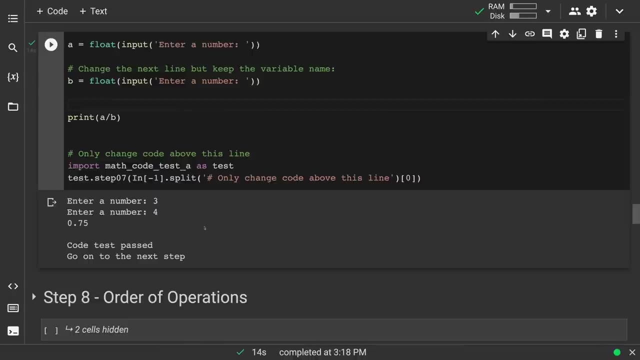 So this is going to work, no matter what somebody enters in, And then when we take a look, then you see it's waiting for us. so I will do enter a number 3, enter a number 4, and .75, which is perfectly fine because they're float. 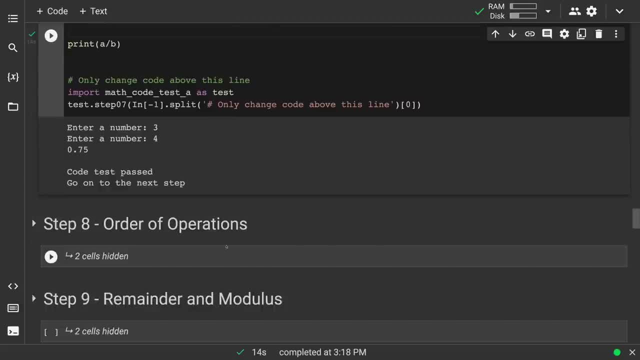 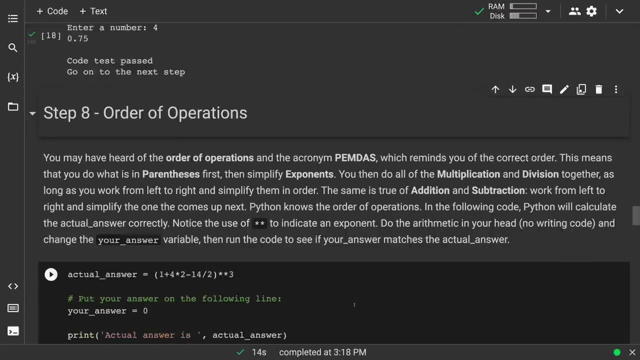 numbers. There we go, Good times, Alright, so order of operations. And yes, Python knows order of operations, So in case you forgot you know, here's the acronym PEMDAS. parentheses. exponents, multiplication and division, addition and subtraction. 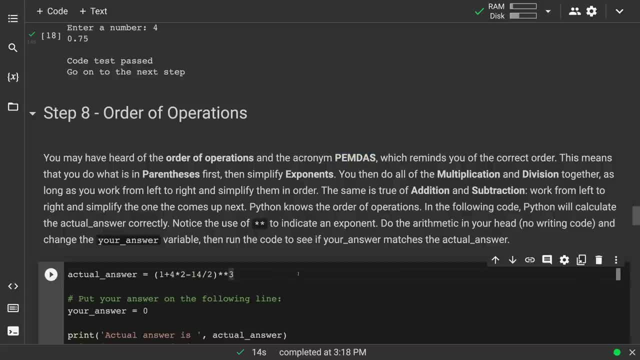 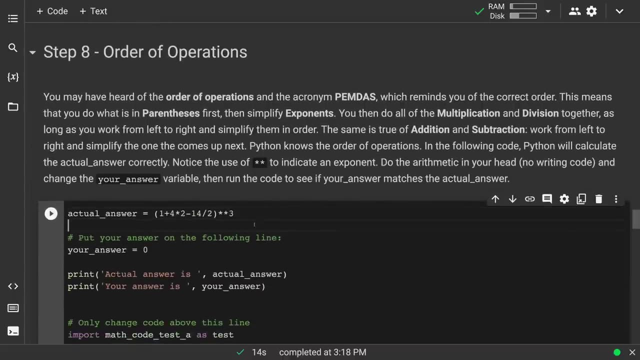 So you could, and then remember: the Python syntax for exponents is the two asterisks. So in this case, what I wanted you to do is test your knowledge of order of operations. We're not even worried about actually writing code here Then. 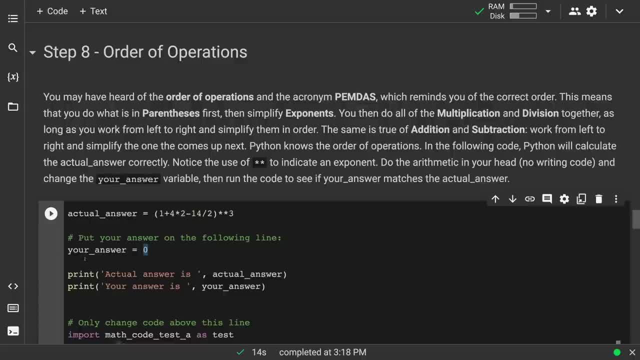 you're going to put your answer here, But don't really think about it. See if you can do this in your head. What would this actual answer be? And then you're going to put that here. Well, you're going to put that here for your answer. 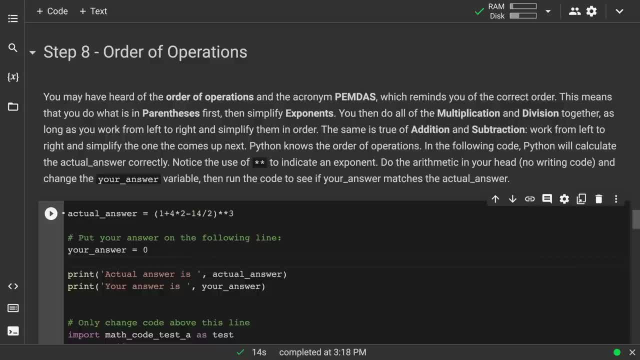 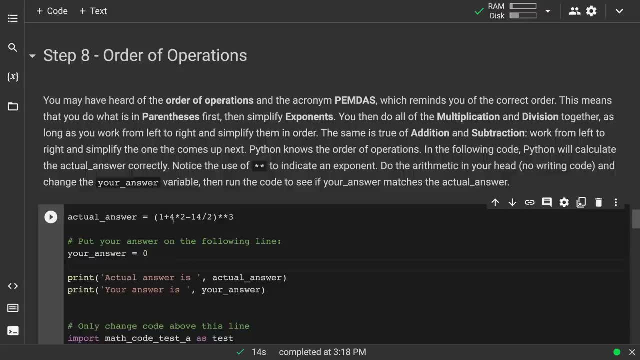 And then, when you run it, Python is going to calculate the actual answer and your answer, and then you'll see. Alright, so let's look at order of operations. Everything in the parentheses first, and then multiplication and division as they come up. So 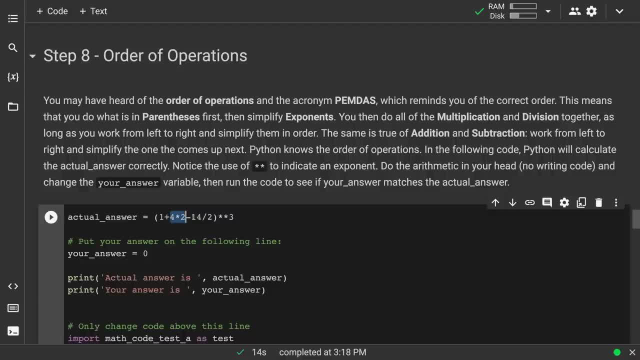 four times two, and then we have fourteen divided by two. So you can actually go back and forth multiplying and dividing all day. So, as they come up, four times two is eight, and then fourteen divided by two is seven. So then we're going to have one plus eight. 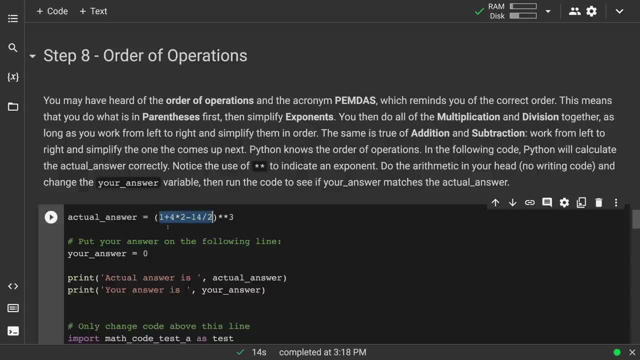 minus seven, And so one plus eight is nine minus seven is two. So then we take two. Now we're done. the parentheses to the exponent Two to the third power is eight, And so there you go, Put your answer in there. 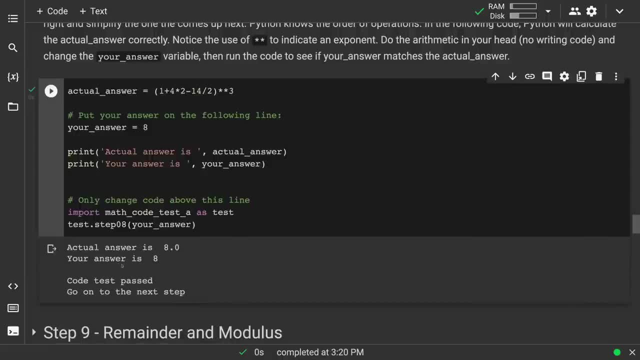 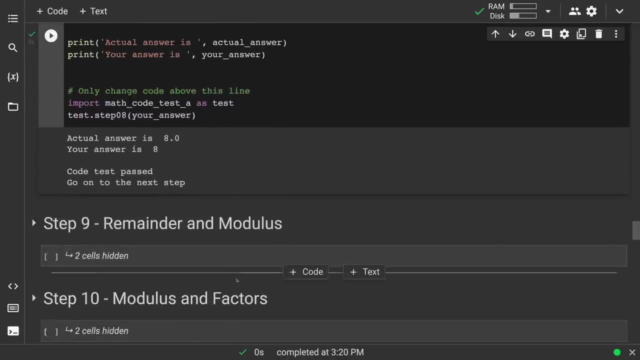 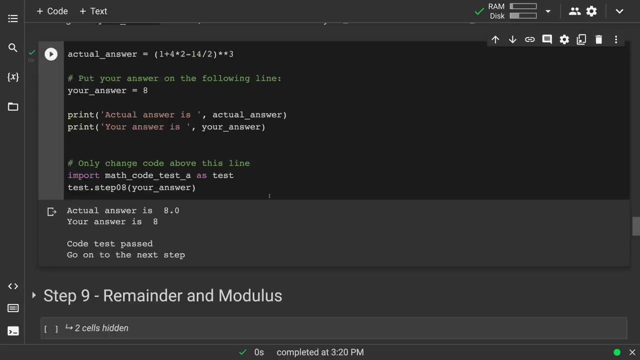 And there we go. Actual answer is eight. Your answer is eight. Code test passed. Okay, so all these things, and remember, you can just like the other ones, you can do all this, You can put print statements, you know. 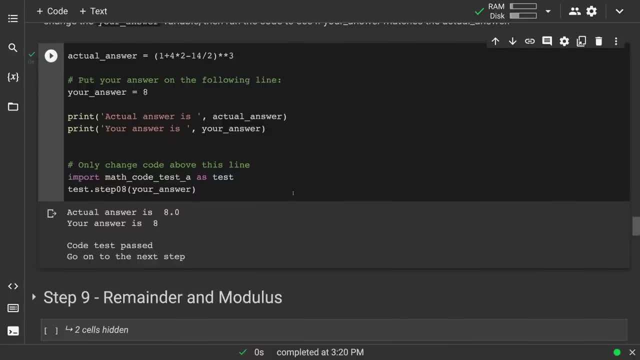 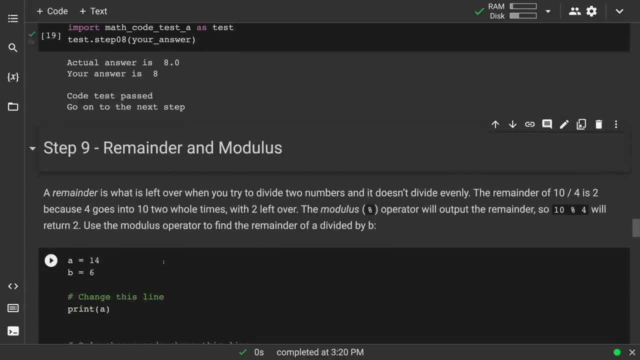 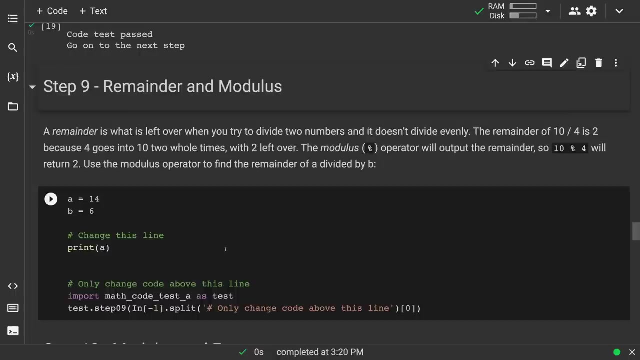 whatever math you want, Just straightforward math in a print statement. Python will do that for you. So those are some simple calculator tricks you can do. Okay, so remainder. Remember: when we divide something that does not work out evenly, we have a remainder And the modulus. 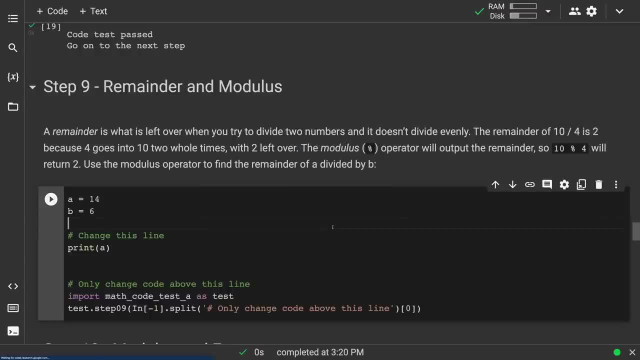 operator looks like a percent sign, but if I'm using it in the code it tells me just what the remainder is. There we go. So, as I have the directions here, ten divided by four is two, but with but as a remainder. So 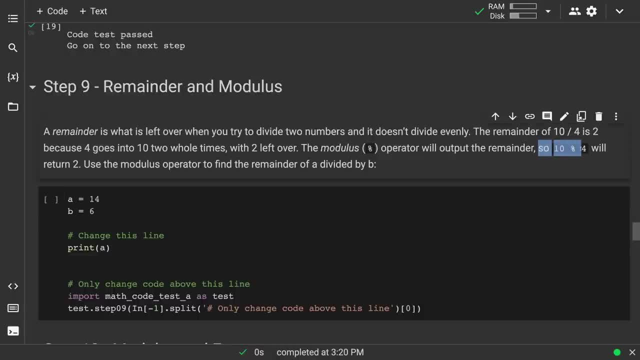 two and then two left over. So ten modulus four would give me two, because that's the remainder. Or fourteen divided by six will have a remainder. So if I do eight a modulus b, and again it's the percent sign, On most keyboards it's on the same key as the five, but you have to hit. 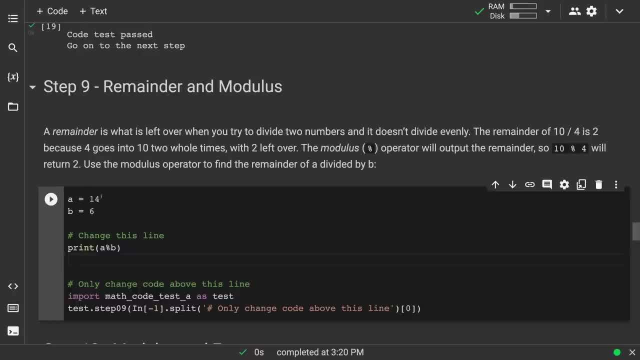 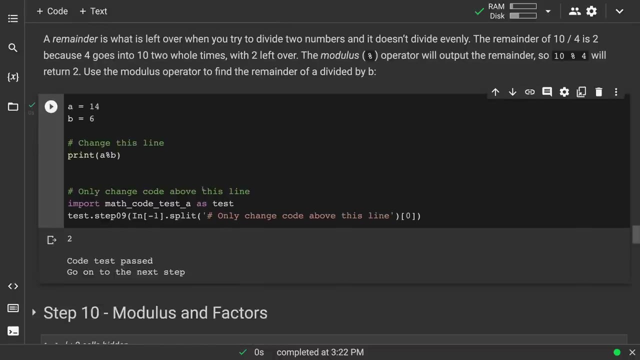 shift. So fourteen divided by six- Now, let's take a guess: Fourteen divided by six is two, with a remainder of two. So that's what we're expecting to see: the printout. There we go Now. actually we could. you don't need to do this, but we could show. 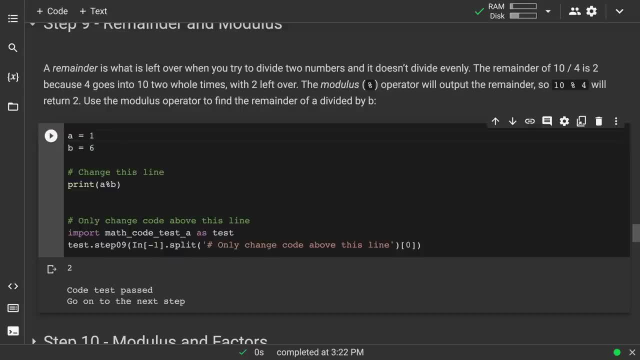 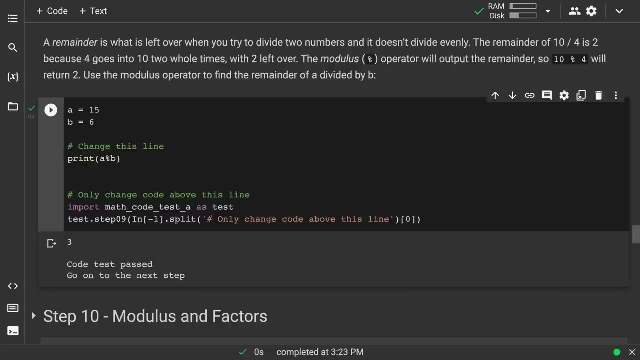 well, supposing if I had fifteen divided by six, So six times two is twelve, so there would be three left over, And so a modulus b would be three. If you wanted to, you can test these out, because this particular code is: 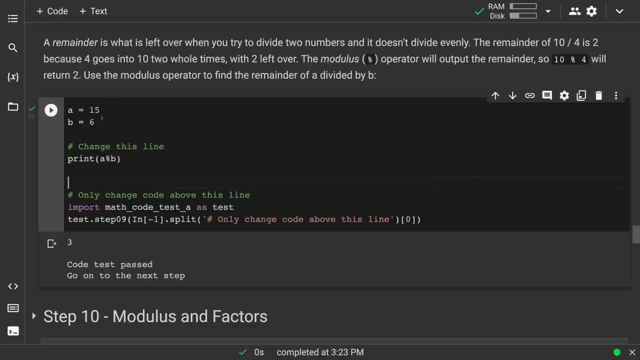 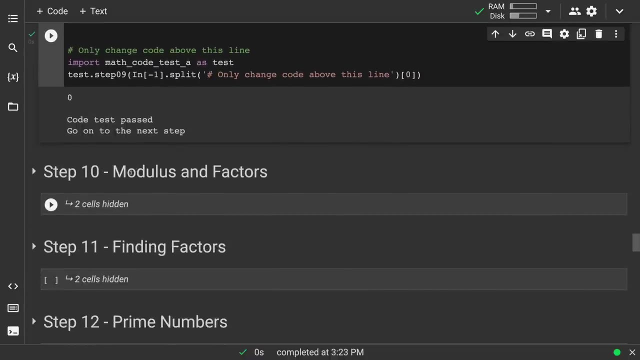 testing? did you do it correctly here? So if you wanted to go back and try some different things, Whereas then if I go to eighteen, that works out evenly, so the modulus would be zero. There would be no remainder, And we can use that to find factors. 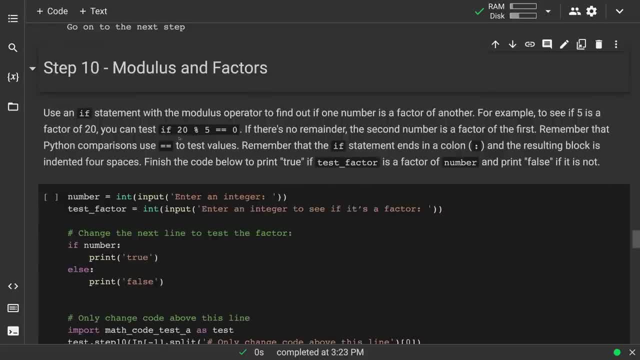 So we'll have an if statement here. So if I have twenty modulus five, so that's twenty divided by five is four, works out nicely. So twenty modulus five, the remainder would be zero. So if that's zero, which it is- 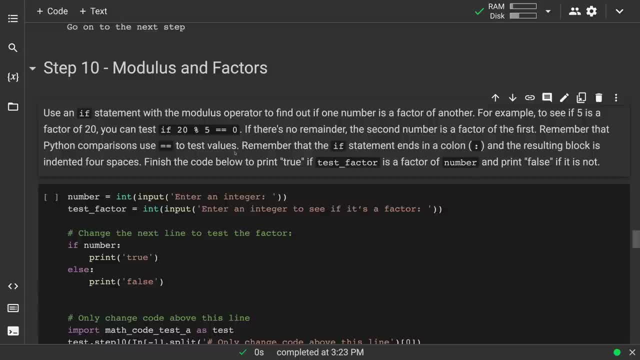 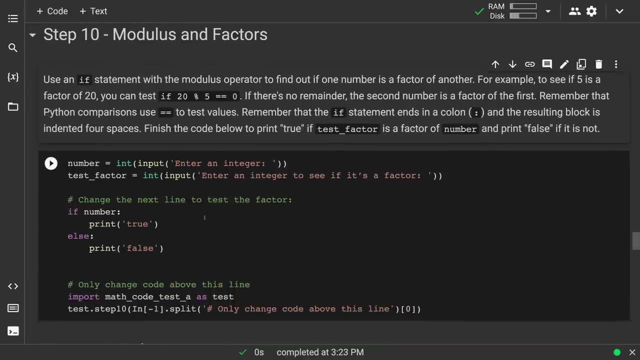 then that means five is a factor. So you see, we're using the double equals to test it. So that's what we're going to do here: We're going to walk through this and we're going to cast. This time we do want integers, because 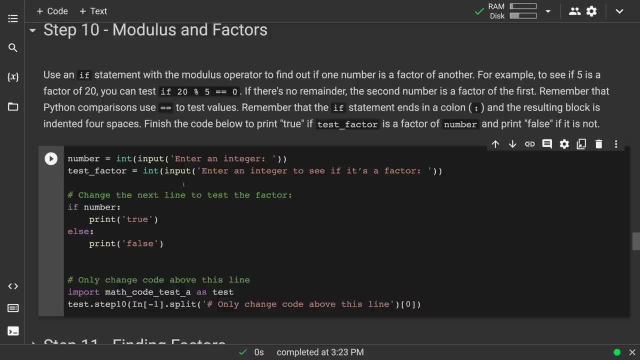 factoring really only works with integers. You know we can divide a lot of things, but you know if it's a factor there's going to be a nice integer in there. So I'm going to just enter an integer, So input cast it as int and that's going to be our number. And then here: 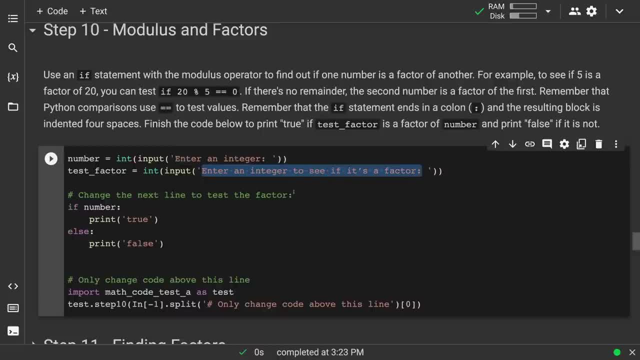 next one: enter an integer to see if it's a factor And again cast that as an integer And that's going to be test factor, because I don't know if it's a factor yet And in the if statement I just have if number. 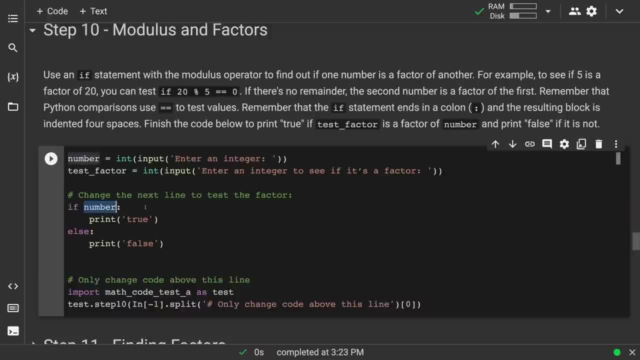 Now remember: whatever this is: if it's true, it's going to do that. So if number exists- which it will- then it's going to do this, But we're going to change the next line. So what do we want? Number modulus. 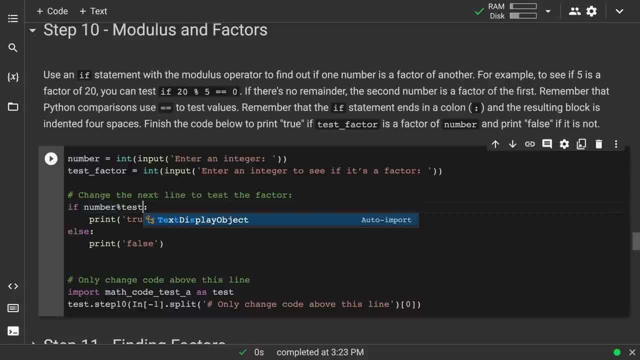 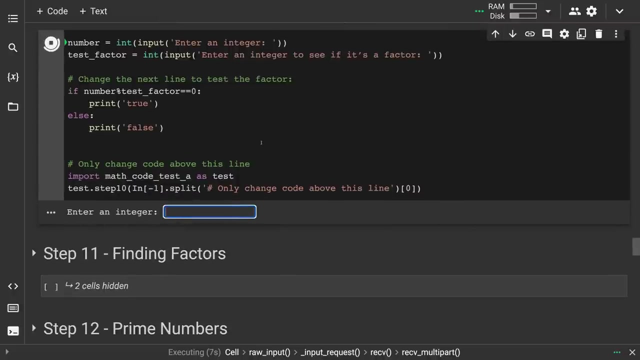 test factor. And then now, if that divided by that gives you 0, then we can say: true, it is a factor, And then or else it's false. So there we go And enter an integer, So let's do one that doesn't work. So if we have 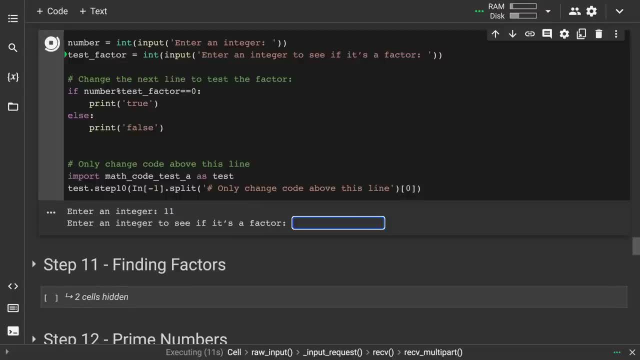 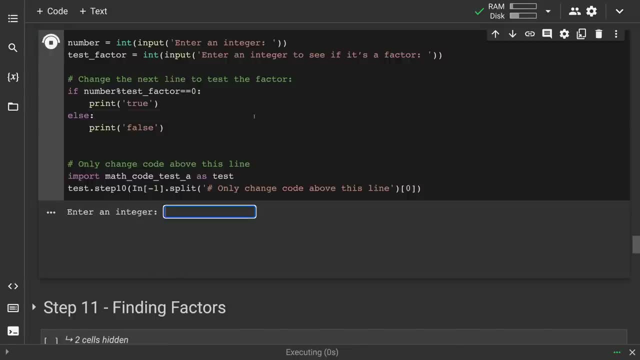 11 and 5, false. And we can run it again And, let's say, make it 12, 3, true. So there we go, showing how we can cast things, and we can use that to test if something is a factor. 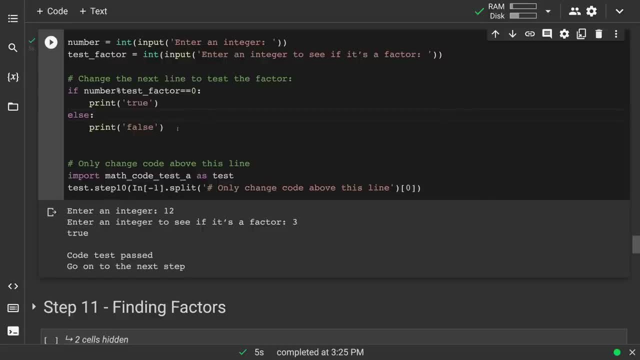 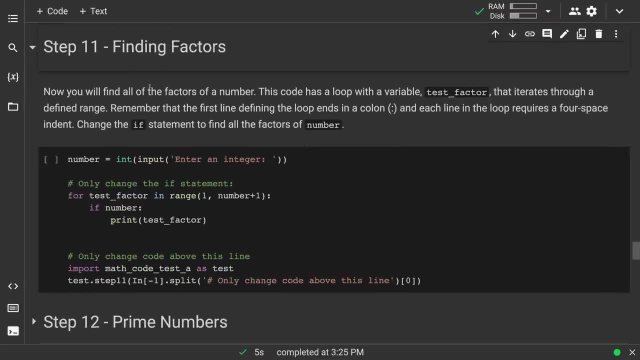 That itself might be useful, but we're going to take that and we're going to build that into other things Like this. finding factors: Alright, finding all the factors of a number. So very similar to what we did, but we're not. 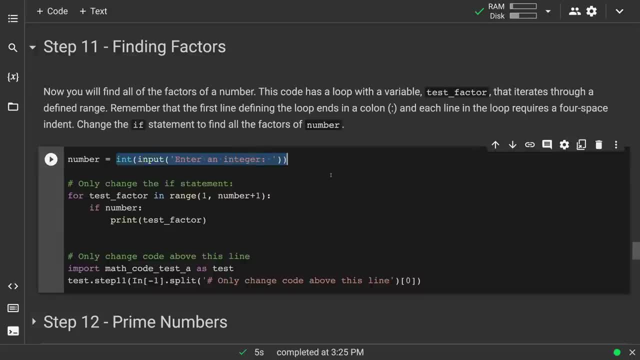 asking for second input. here We have the first input and then we want to find all the factors. So now I have my for loop for test factor in range. So I'm going to take this range. Let's look at this backwards here. I'm going to take this range and if I just had one number. 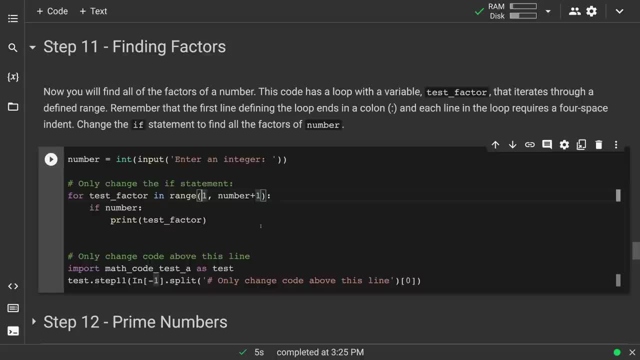 in there it would start at zero, But I can't have that because that'll give me a divide by zero error right away. So I'm going to start the range at one and then end the range at number plus one, Because normally the range it won't do that last. 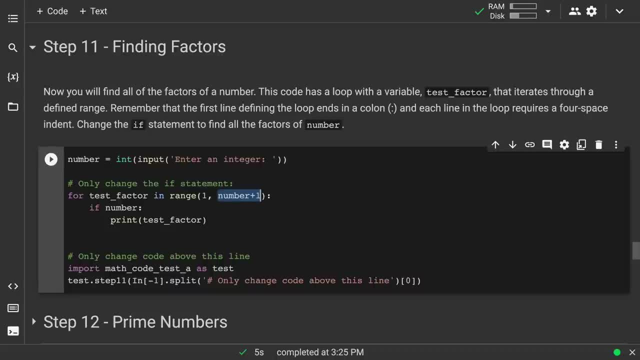 number. So I have to add one in now to make sure. Whatever that number is, I want to include that. Alright, so now for test factor in this range. it's going to loop through every number in this range And one at a time. 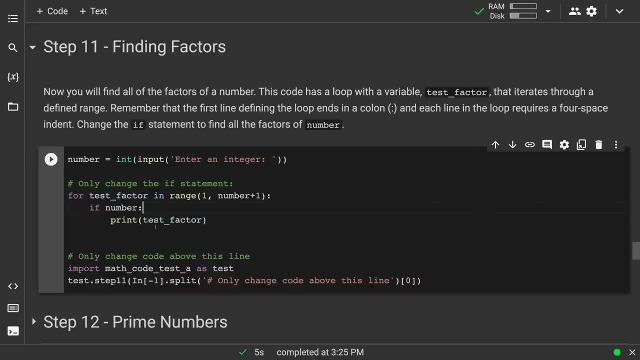 test factor is going to be one And then the next time through the loop, test factor is going to be two, So it will just loop through for that many times For every number in that range. Alright, And this is where we're going to change the if statement. 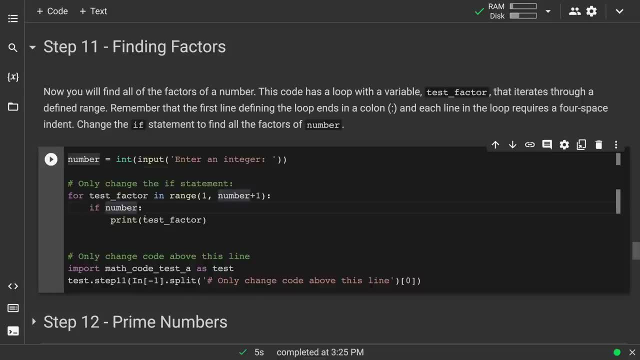 So we want to say: if it's a factor, So number is the original number we want, And each of these test factors, what do we want to do with it? We want to say if number modulus test factor equals zero, Just like we were doing. 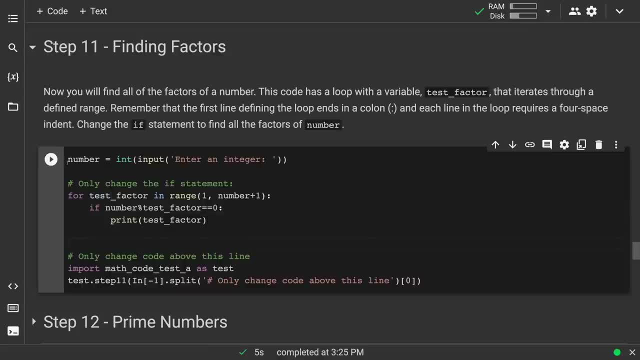 before. we were just kind of putting it in an if statement now. So I get this number and I'm going to loop through all these factors from one up to that number, And then if number divided by test factor gives me a remainder of zero, then it is a factor. So then I'll. 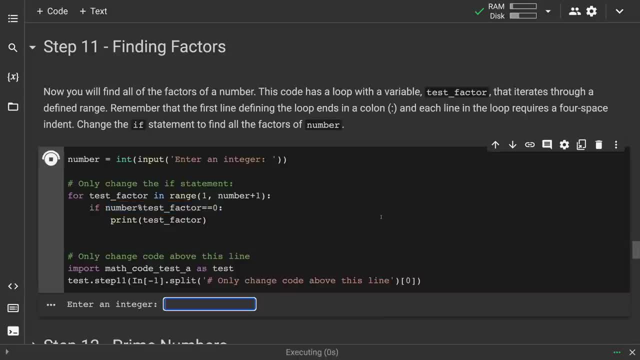 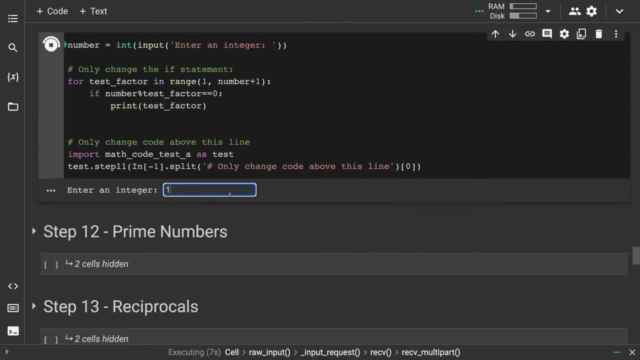 print it out. Alright, so we run it and what do we have? Let's say, twelve. Twelve is a lot of factors And you see, it will print them all out: One, two, three, four, six and twelve. 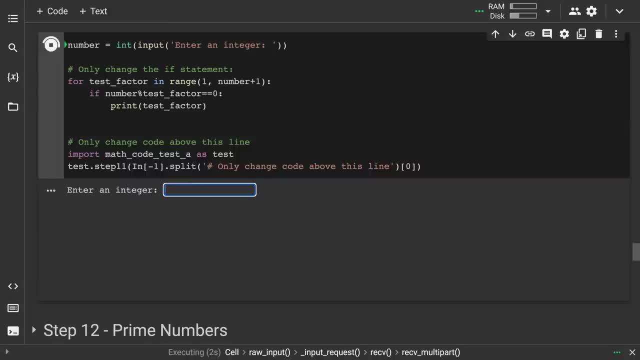 And we can run it again. Enter an integer, Supposing I enter like seventeen, One and seventeen Because it's prime. So that's what we're doing, Just showing all the factors here, This type of thing. we will revisit this at another. 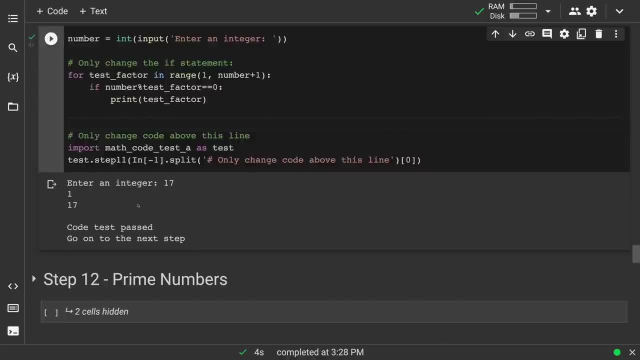 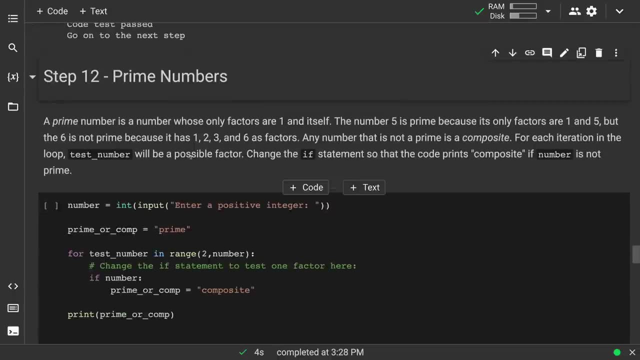 time to reduce fractions to lowest terms. Okay, Now what about prime numbers? So a prime number is a number that the only factors are one in itself. So we're going to, and then anything that's not prime is composite. So, if I have 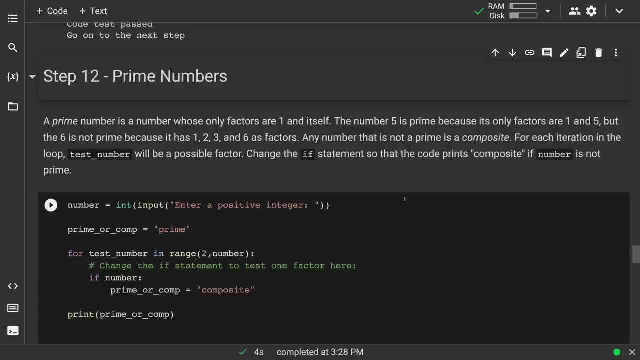 you know, five is prime, because the only way you can multiply to get there is one times five, But six as one you can do one times six, but you can also do two times three. So because you have those other factors, it's composite. 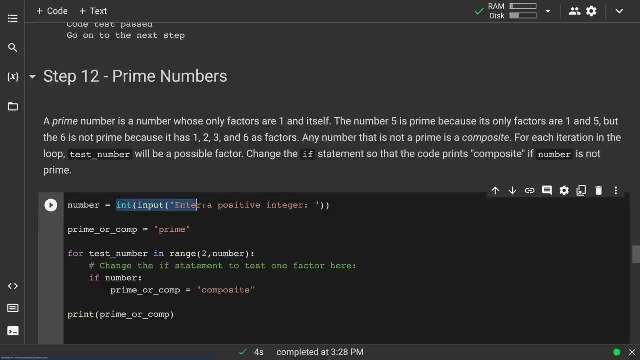 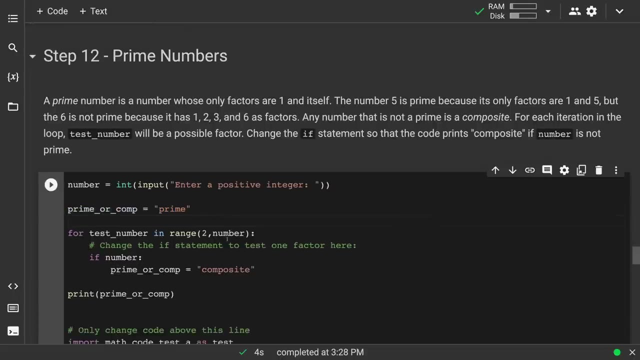 So here now we're going to have same input and again integers, because we're looking at factors, And I'm going to start out with this variable, prime or comp, Say it being prime, And then same thing, range. Now notice I. 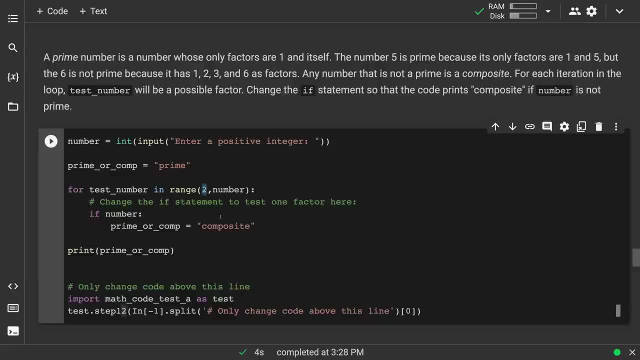 started the range at two, because one will go into everything and that's not what I want. That won't tell me anything. So I'm going to start at two, up to and including the number. Again, not including the number, because this time 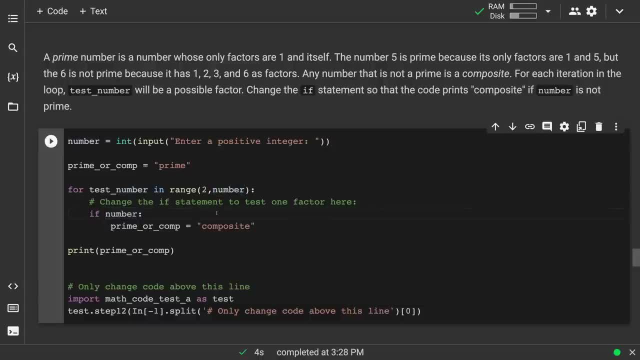 it won't include the number. I didn't add the one there because- again same reason, I didn't have one One and the number itself. yeah, we know that those are factors, But I want to find out from two, through any of the other numbers, if it's a factor. 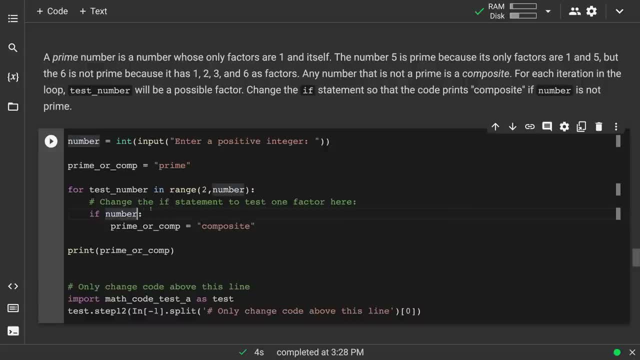 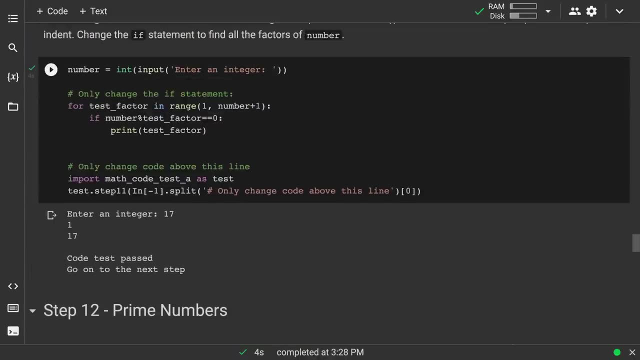 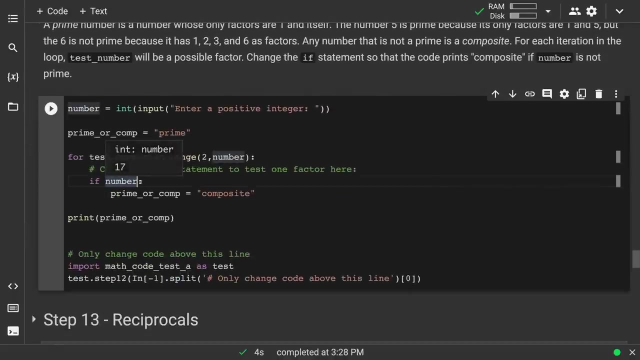 And very similar, then if number, we're going to do the same loop And you could always go back. if number divided by test factor equals zero, There we go, Because we have the same variables here. Always double check just in case the variable names change, or it's a slightly. 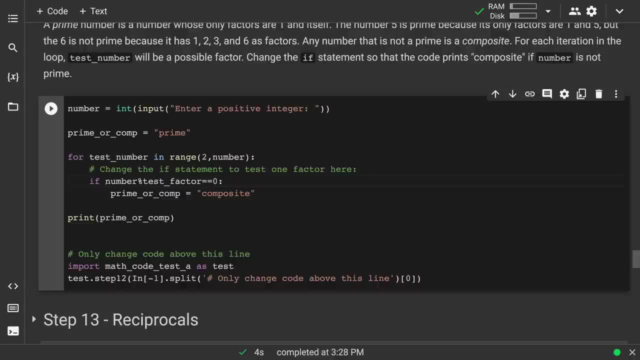 different way of doing things. But yes, if that test factor works. oh see, because this is test number. So this would have given me an error. And that's the thing with reusing code. yes, we know we're all going to use a lot of copy and 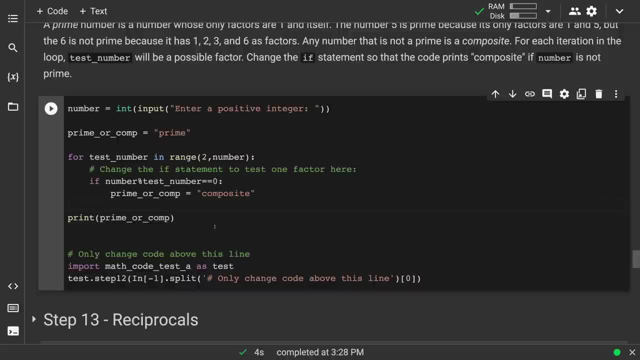 paste because that helps you know if it's a whole block of code, But be really careful that it is exactly the variables and everything that match up correctly. So you know, a lot of times people do too much copy and paste and 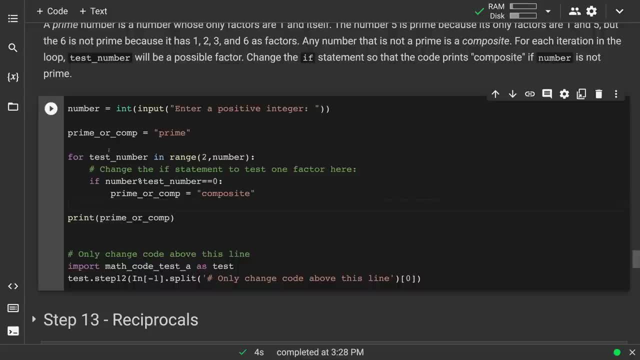 then they're lost because things don't match up. So this one we call it test number. So if number divided by test number, if that has a remainder of zero, then that means that is a factor, which means all it has to do is happen once. 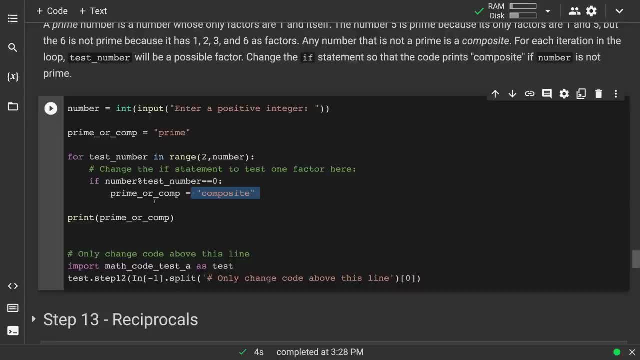 and that means the number is composite. It's only prime starts out. that variable is prime and it stays prime only if it goes through, and we never get a factor here throughout the entire thing. Alright, so let's take a look. If we have 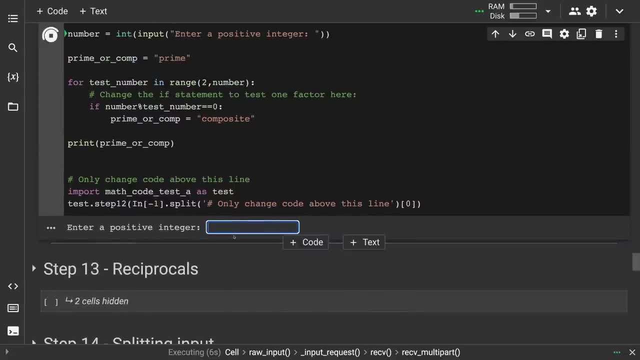 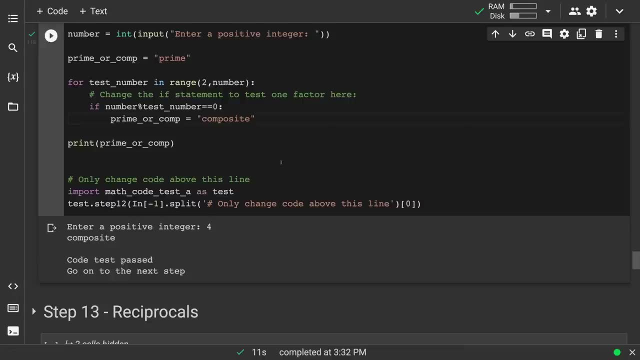 this and enter a positive integer. So let's enter one, let's say four composite, right, Because I can also do two times two. And then let's enter one that we have seven prime, And that way you can check all kinds of other things. 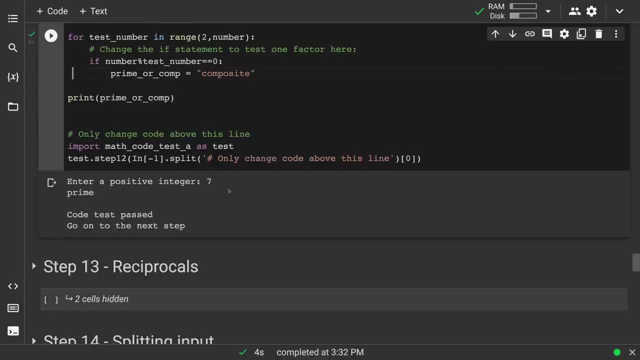 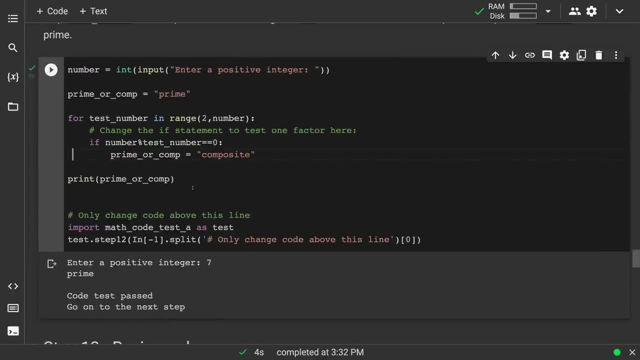 You know, oh, some huge number. is it prime? is it composite? There we go And you know, now that you have this, you don't have to change any of the code when you run this it'll, you know, it'll. 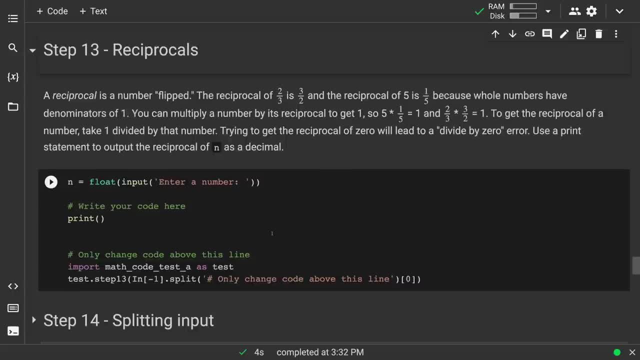 test it for you. Alright, other interesting things: reciprocals. So writing it in math it's the number flipped. So I have this: reciprocal of two thirds is three over two. You see it just flipped. And then any whole number. the reciprocal of five is one fifth. 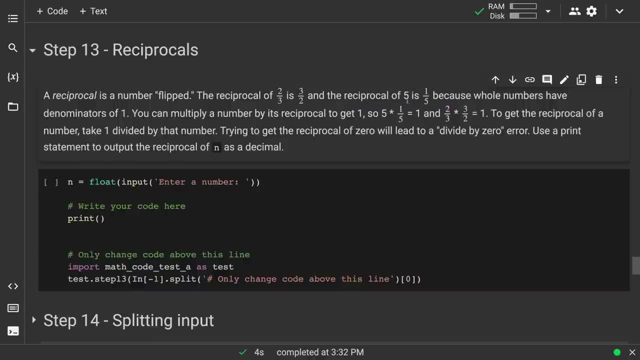 because any whole number, it's understood that it's a denominator of zero Or, sorry, denominator of one, So that'd be five over one. So then that's why it's one fifth as the reciprocal, And you can multiply a number by its reciprocal and get one. 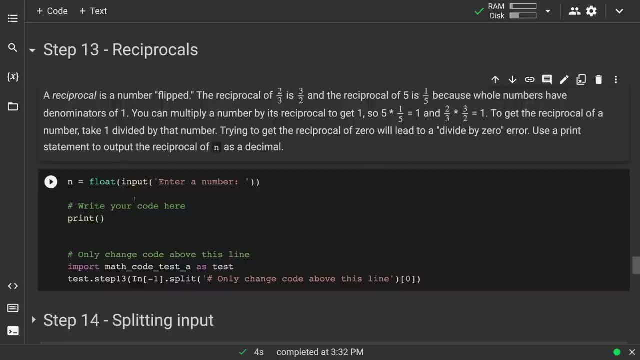 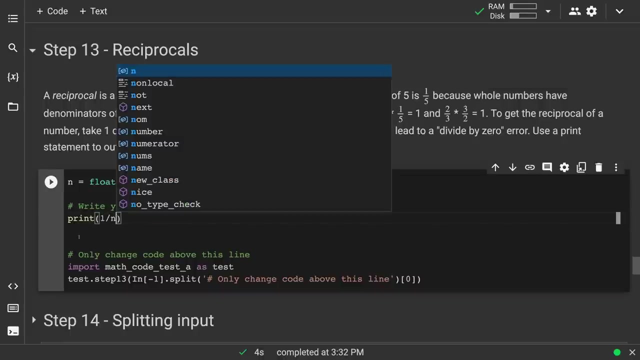 There we go. Pretty good, So, and there we go. Zero has no reciprocal because it'd be divided by zero. So we can write the reciprocal whatever the number is. we can just actually flip it: One divided by n. That's actually all you need to do to find the reciprocal. 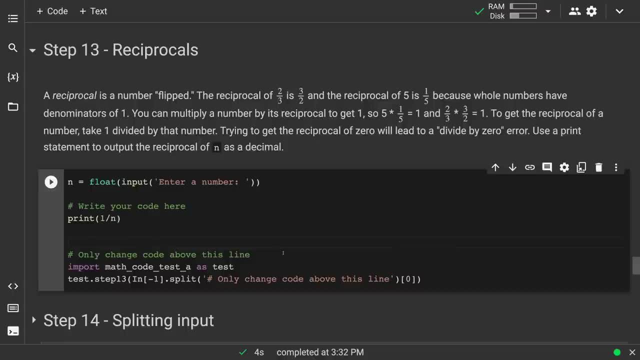 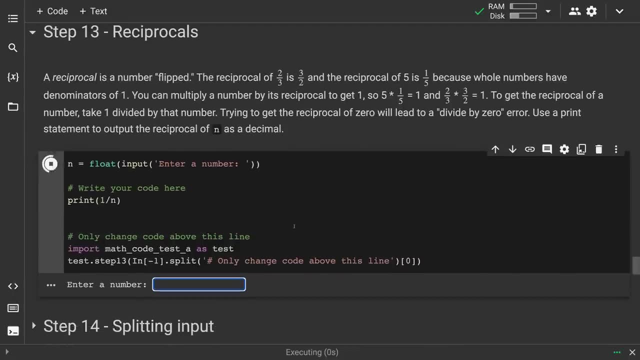 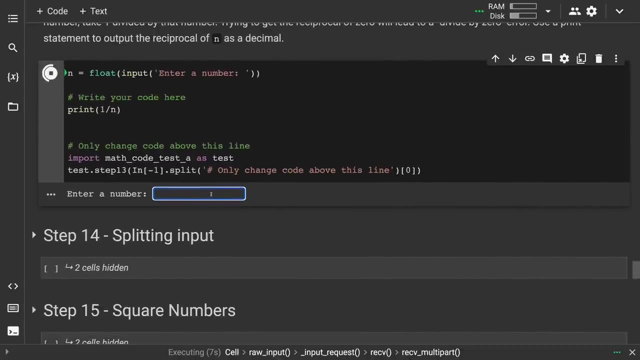 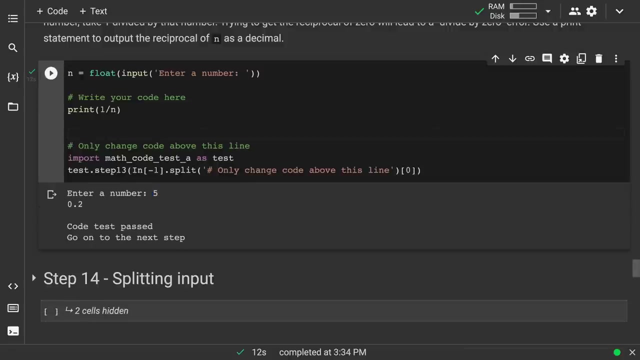 And some of these might be decimals, but nonetheless this will find the reciprocal for you, And we see our output here. Enter a number. and what if I have the number as five? See point two. but that's the decimal equivalent of one fifth. 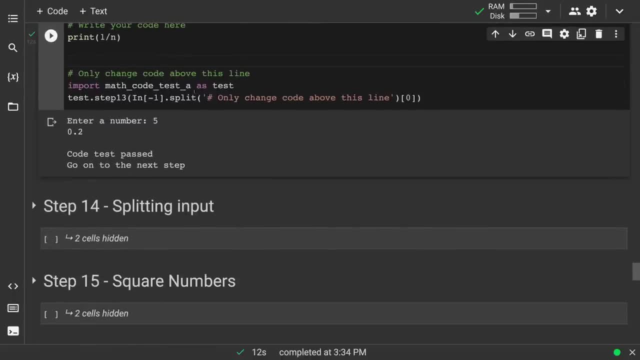 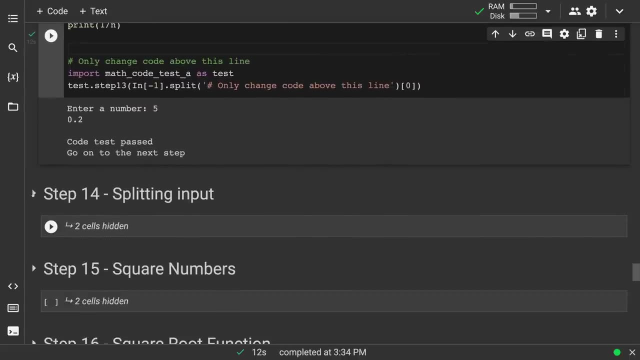 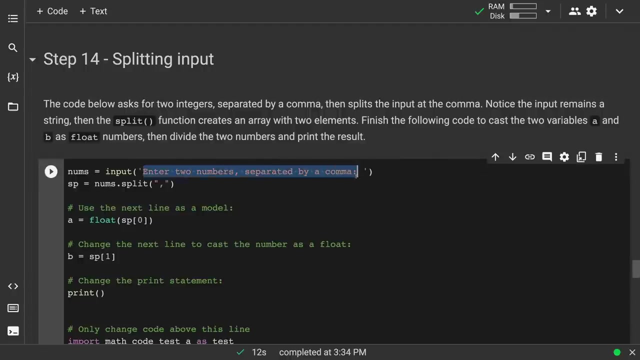 Alright. So just putting this in there, showing you what you can do with finding reciprocals. Other things we can do with the input is supposing I wanted to have an output like this: Enter two numbers separated by a comma. Oh Well, 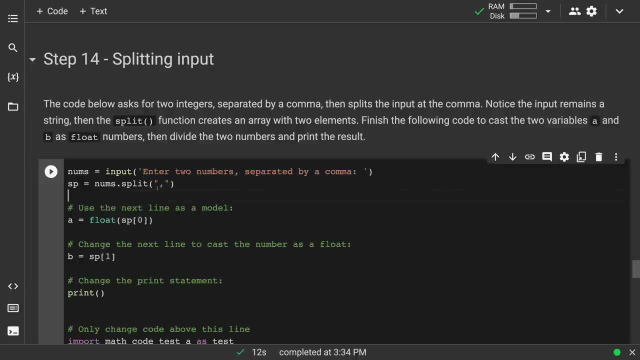 now. but I want to test each of these numbers so I can split it. So this, I'll store it as the variable nums. Still didn't cast it as anything. And then here this is actually going to be an array, in this case with two elements. It's going to split it at. 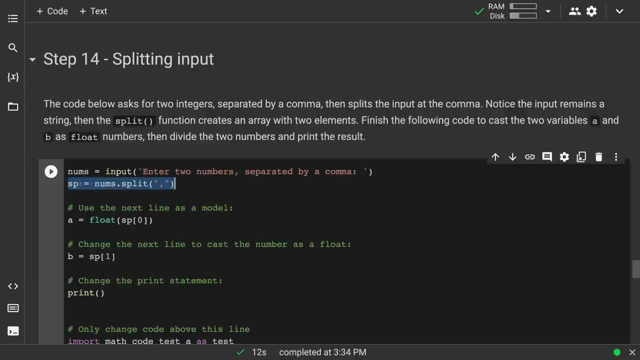 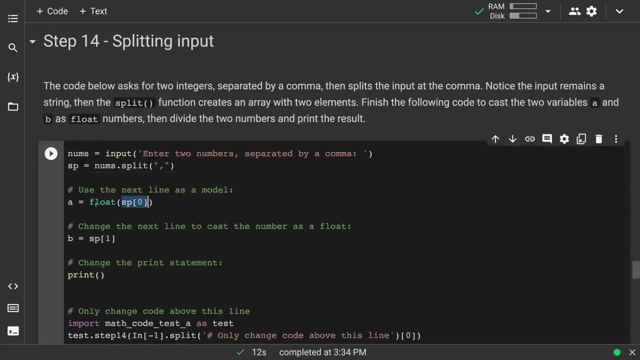 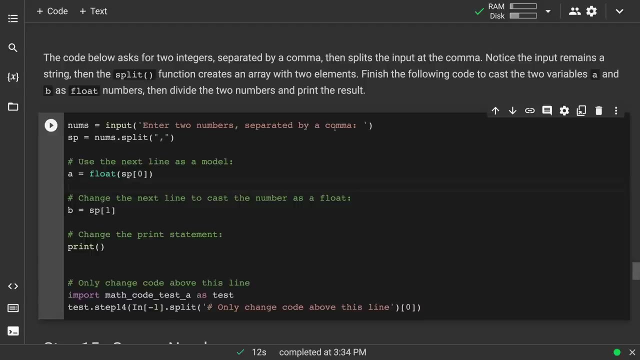 the comma. And then now this array sp has two elements. So I have sp0, the first one. I'll cast that as a float, And then I have sp1.. So that's it Asking for it to be separated. 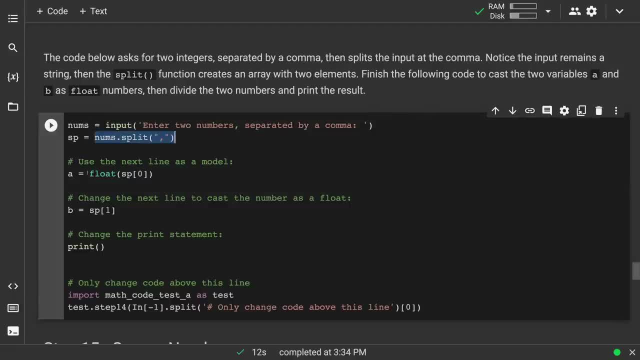 by a comma, Split the input And then cast each of them separately. So sp0 and then sp1.. And notice, the code here just says: cast it as a float, So float. Remember to close the parentheses over here. There we go, And then what do we? 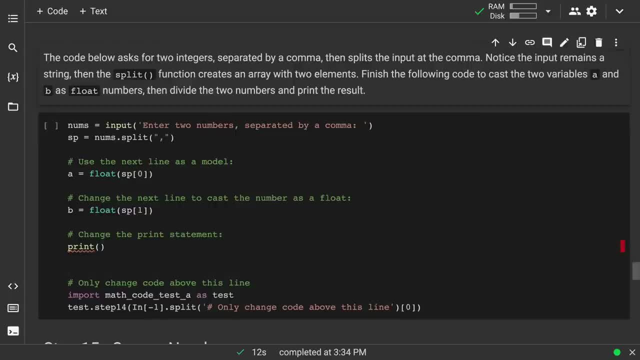 want to do. The directions here are: then divide the two numbers. So that's why we cast them as a float. Divide the two numbers, and we have a divided by b. Alright, So there we go, Split it, Cast it, And in this case then we're going to divide. 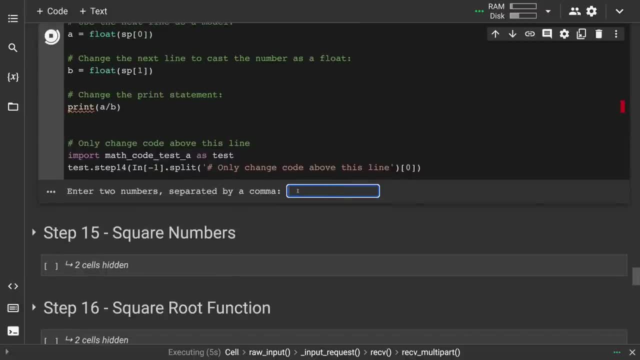 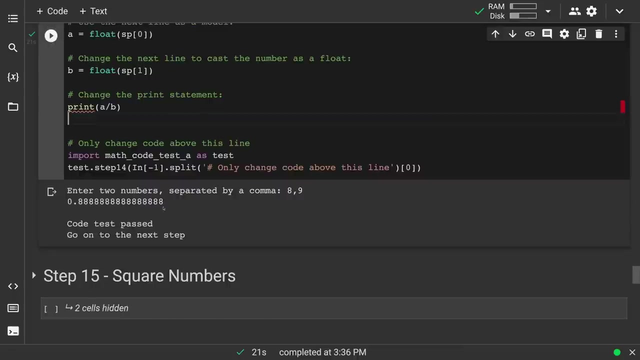 Okay, So enter two numbers separated by a comma And let's see how about we do this. one will be a repeating decimal. Eight comma nine. There we go And notice if you have just one number repeating the fraction. 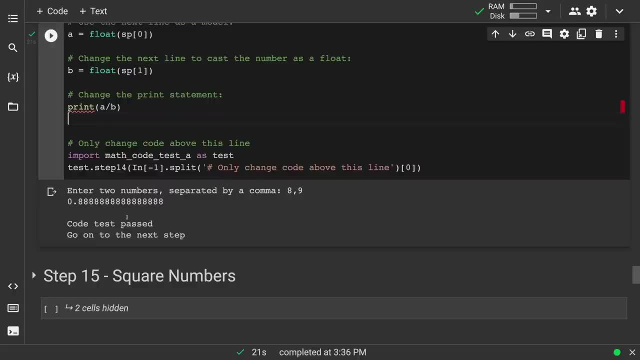 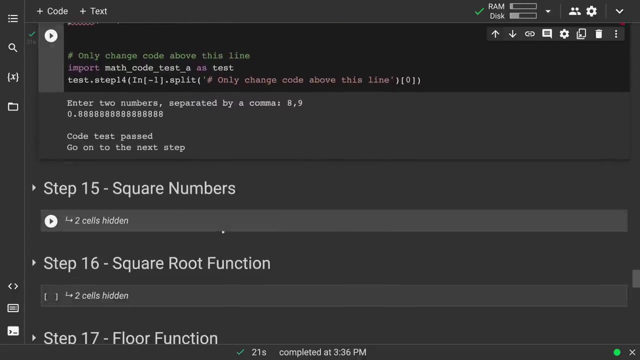 equivalent is that number over nine. So point one repeating would be one ninth. Point two repeating would be two ninths And this one eight over nine. So there we go. Okay, Now, this is building up to something here. 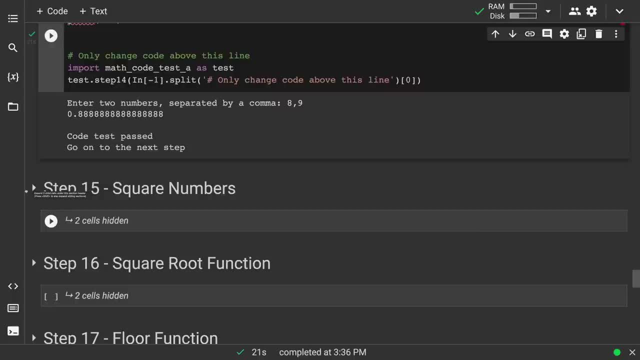 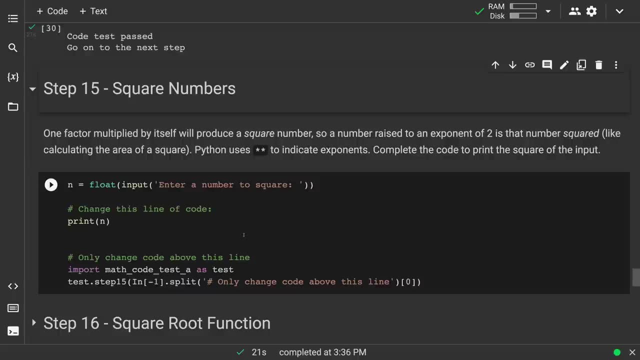 Is building up to you being able to factor square roots. But let's talk about square numbers first. So factor multiplied by itself is a square And it is kind of like the area of a square. You know both sides would be the same. 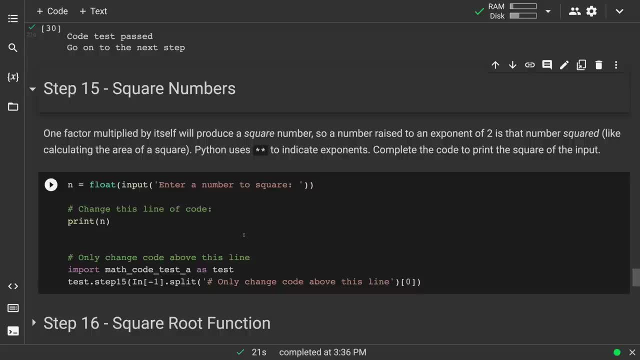 Or all sides would be the same. So when I do length times width to get area, they're the same, And so it's that number times itself, And we would use the exponent as that to the second power. Okay, So all we're doing here is: 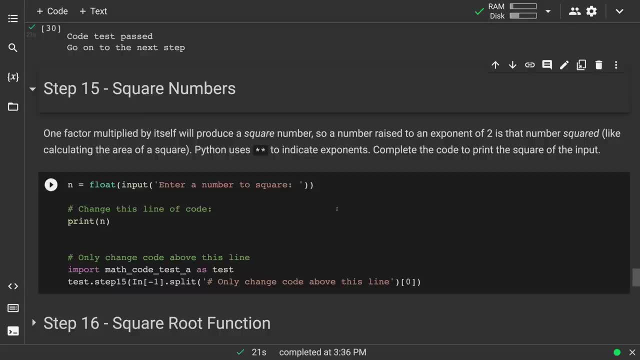 you know we're taking number and then getting the square. So in this case it's going to take the input as n and we're just going to square it. There we go. Okay, There we go. Number to square- Alright Five. 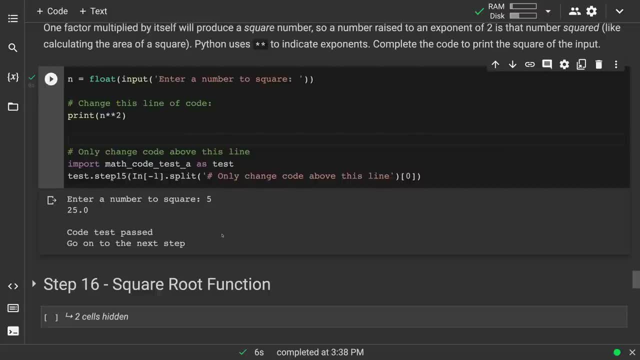 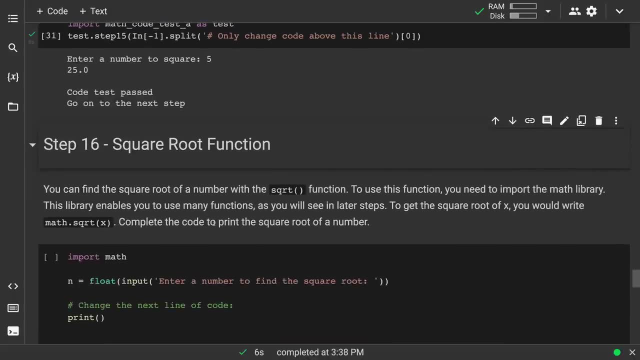 Output twenty-five. Okay, So let's go the other way. Square root function. So anything to the second power, it's squared. But what if I knew the result and I wanted to square root it, So if I knew the area of my square yard. but 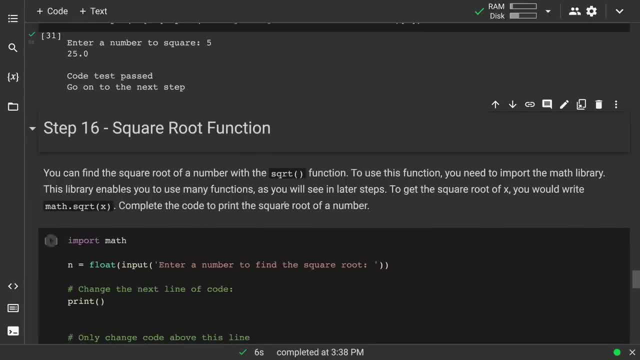 I want to know what's the side measure. So we have sqrt, and that's the first thing we're encountering here that is not built into Python. So we have to import the math library, And this is where Colab really helps you out, because a lot of times you might have to go. 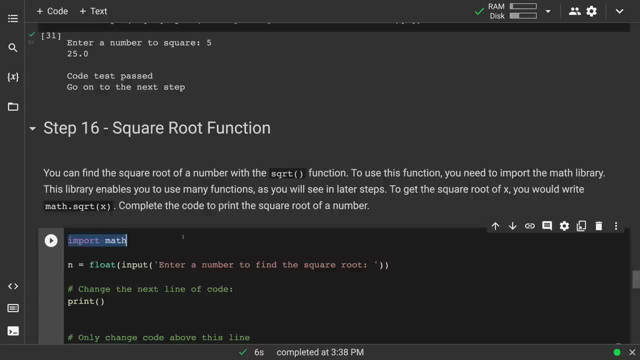 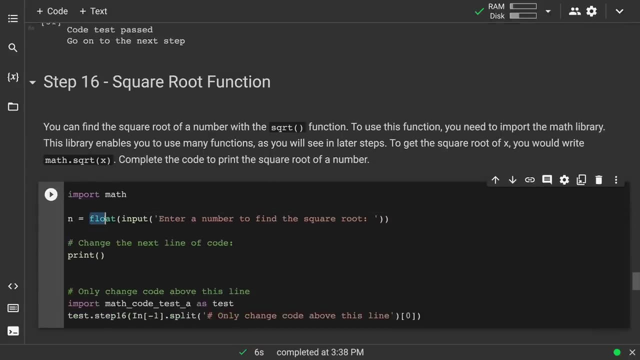 through some other things to install things you know in other notebooks, The Colab notebook, import math- and behind the scenes it works. You just have to have the import statement, Alright, So a number to find the square root Definitely going to cast as a float. 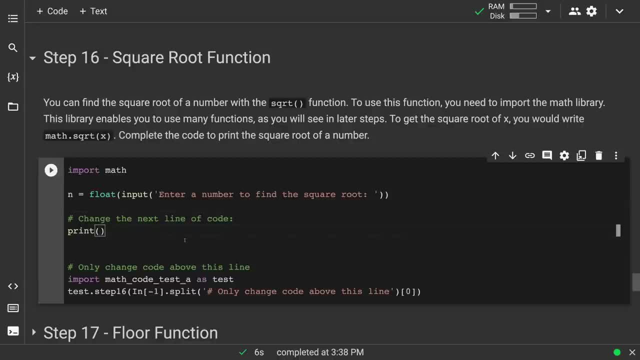 Alright, And how do we get the square root of that? Once we import it, it's going to be mathsqrt and we call it a number n, Especially. you know, even if things don't come up automatically, just you make sure. open parenthesis, one, two, close parenthesis. 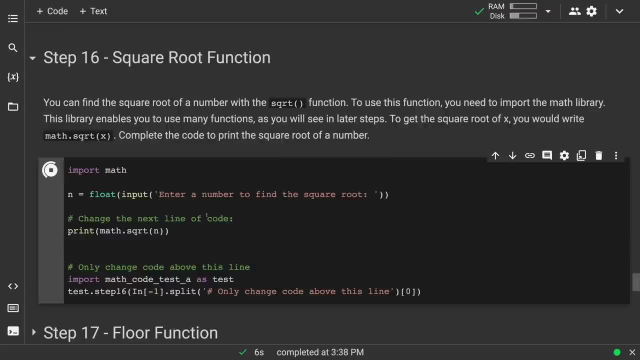 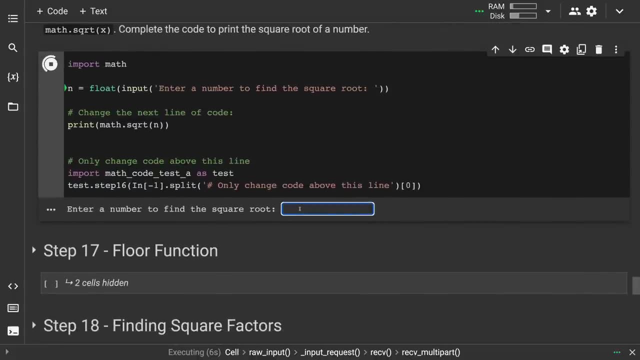 one, two, We got it. So we're going to enter a number and we see here: enter a number to find the square root. So we'll do one that works out evenly. How about sixteen Square root's four? And we can do another one that doesn't work out evenly. 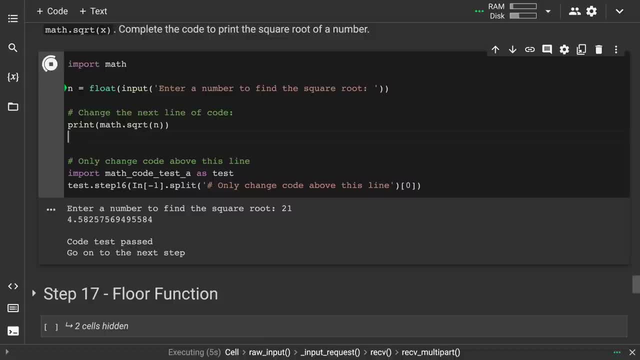 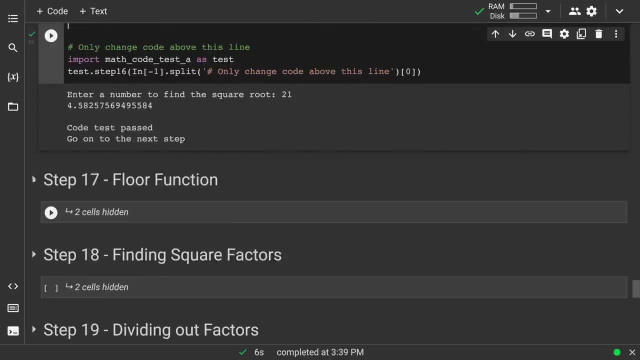 How about twenty-one? And it'll give you a bunch of decimal places. I didn't remember, Yep. So four point five. Yeah, about There we go, Okay. Other cool functions: The floor function. This is another one. We have to import math to use it. 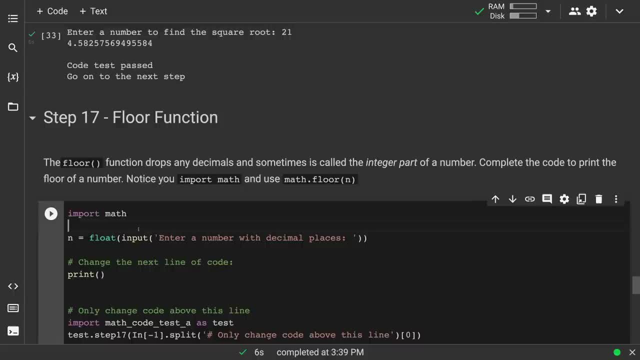 So the floor function. So we have the floor function which just drops any decimals. There we go: Drops any decimals and sometimes called integer part or the greatest integer. So even if it's like three point nine, it's going to drop and just go down to three. 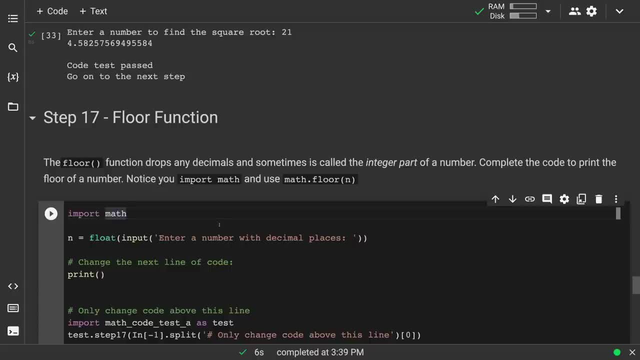 We have the floor function, We have the ceiling function which, as you can imagine, if floor drops all the decimals, ceiling is, no matter what decimals are, even if it's point one, it goes up to the next number And then round the one we use. 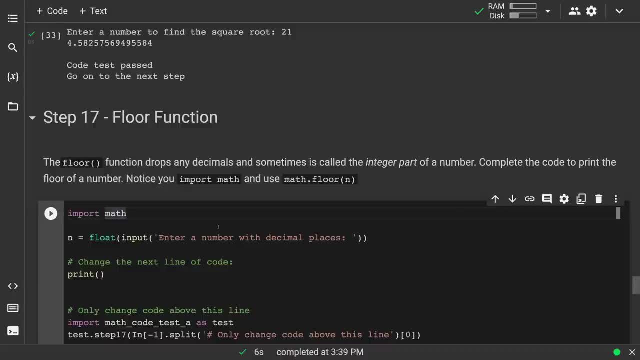 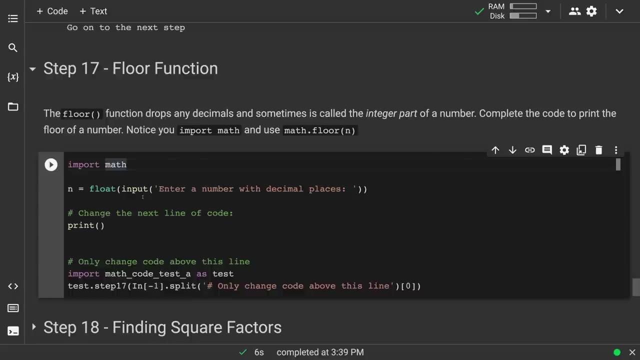 possibly most often round. remember: point five and above rounds up and point anything less than point five. Point four and down Rounds down. So we're going to look at the math dot floor function here. Alright, enter a number decimal place and we're just going to practice doing the math dot floor. 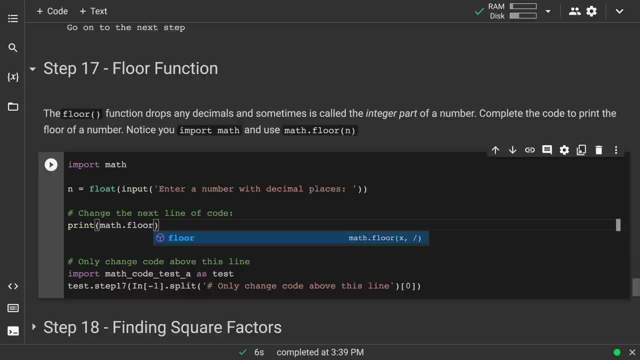 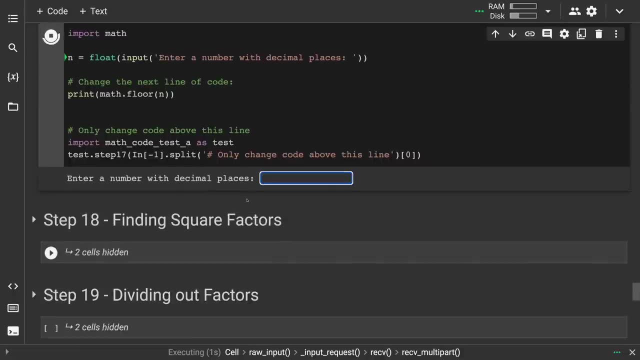 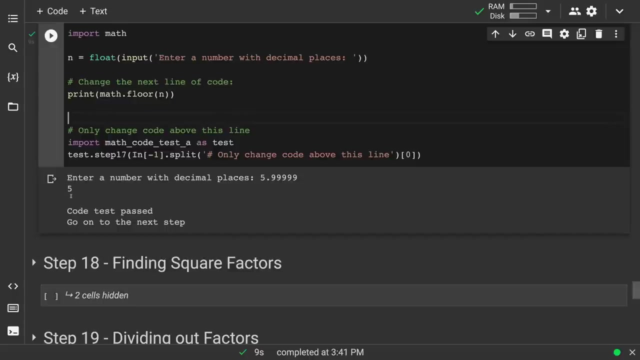 function here, Math dot floor of n. So enter a number with decimal places. So I'm going to call it five, point nine, nine, nine, nine, nine, and when I hit enter yep, and that's the floor function. Even if it's point nine, nine, nine, it drops down to five. 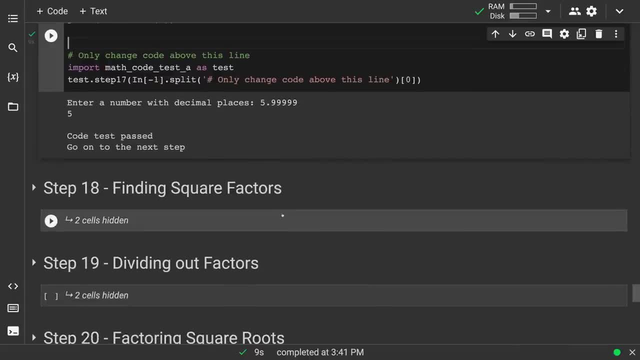 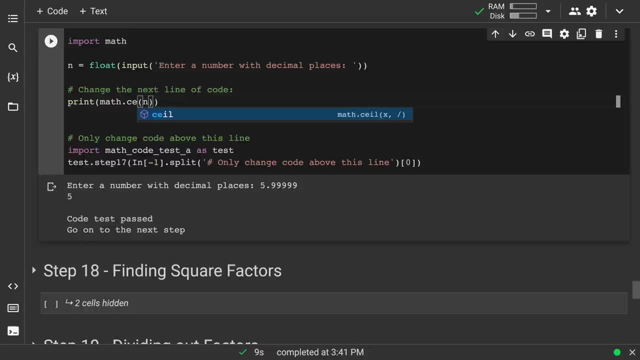 So there we go And remember. supposing you went back and said: oh wait floor, you know I'm upside down Ceiling function. Supposing I wanted to do that, Then alright, so seven point one, because that should round it up to eight. 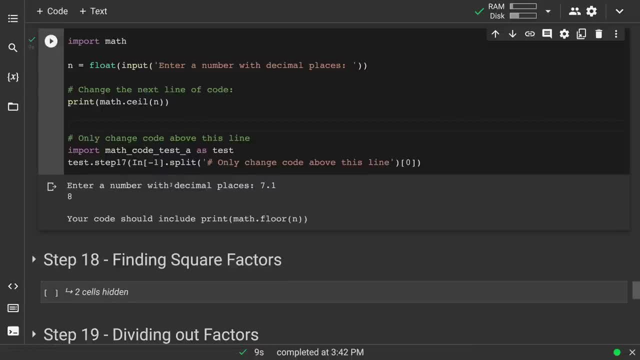 And so that code works. but because that wasn't what these directions are, it'll tell you: oh, you should include math dot floor. And again, if you end up trying different things, it doesn't prevent you from going on. 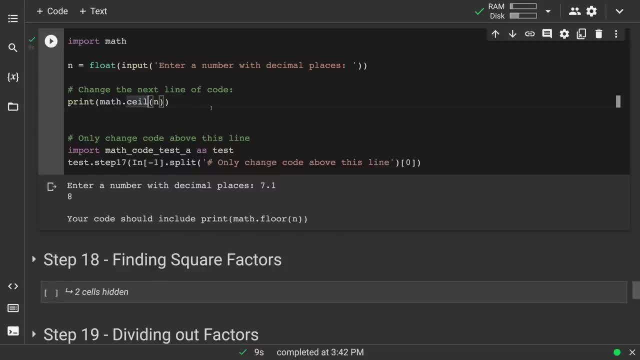 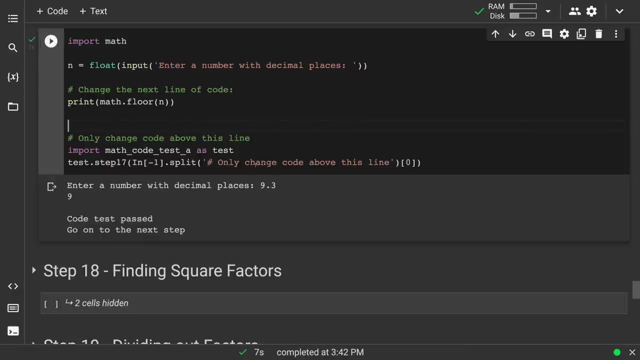 but if you know- I don't know if you spelled it wrong or something or you did something different- it'll tell you: There we go Floor and we go nine, point three: Alright, Good, Drops it. Okay. so 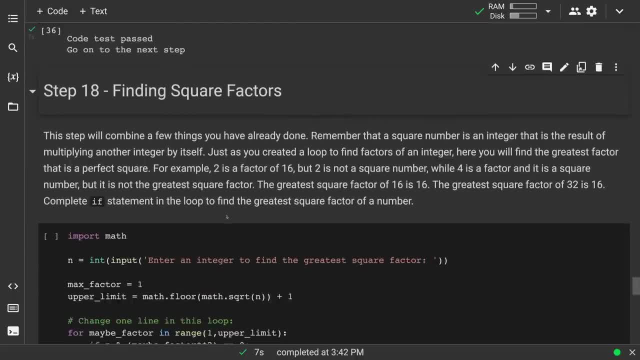 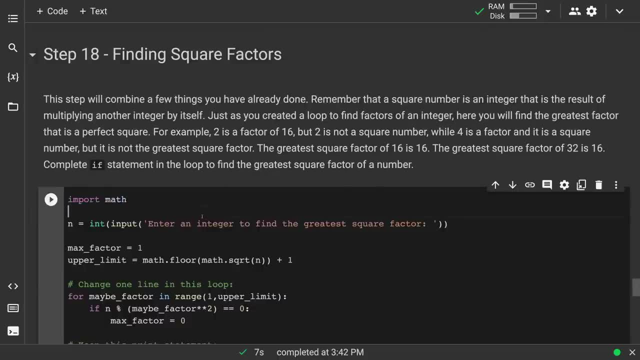 we're going to put some of this together: finding square factors. Alright, so a few things we've already done. We're going to import math and what we're going to do is we're going to enter an integer to define the greatest square factor. 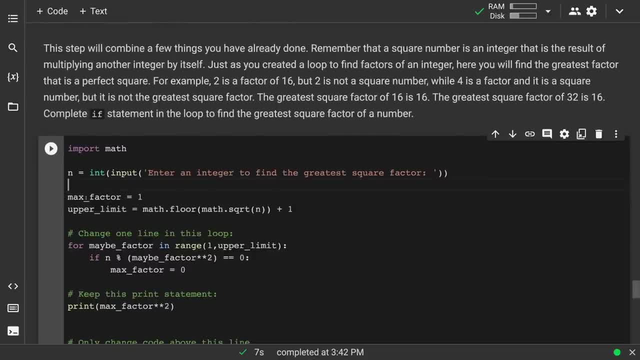 So I'll call that max factor, and right now it'll be one, And then the upper limit. so notice, we're stacking on these functions here, The math dot, floor of math dot, square root of n, but then we're going to add one to it. So 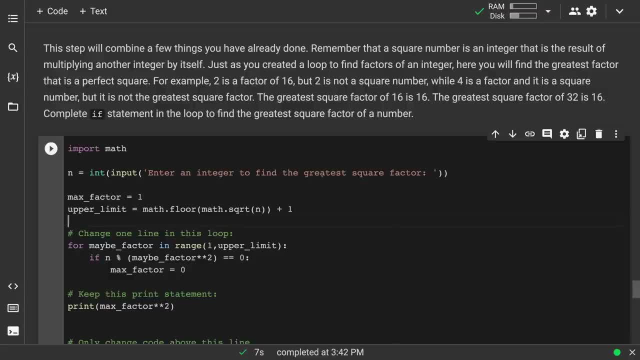 we want to find the greatest square factor. So whatever number you enter it in, we're going to square root it. That's going to, of course, have a bunch of decimal places, and so we could do the math dot floor and then add one to it. Now. 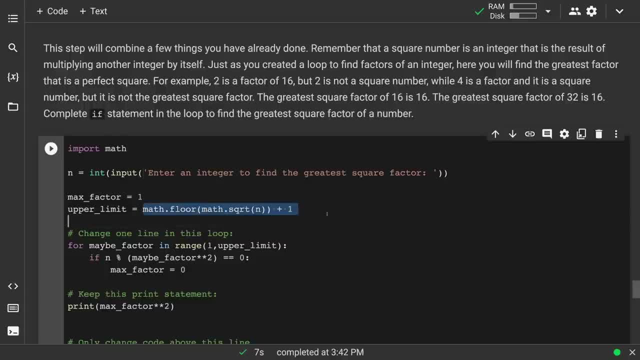 I realize that I could have just done math dot ceiling and then skip the plus one. I, for whatever reason, I did this. I like it, so I kept it. But there we go. That's why, Yes, uh, so that. 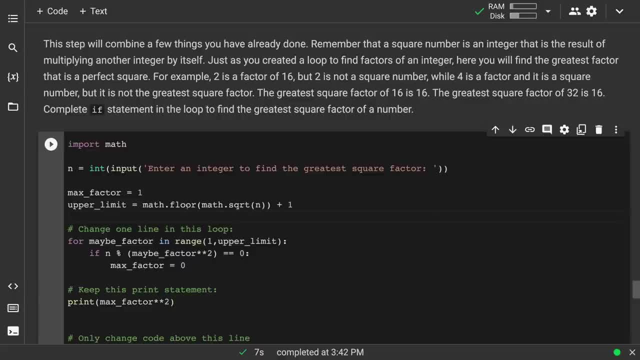 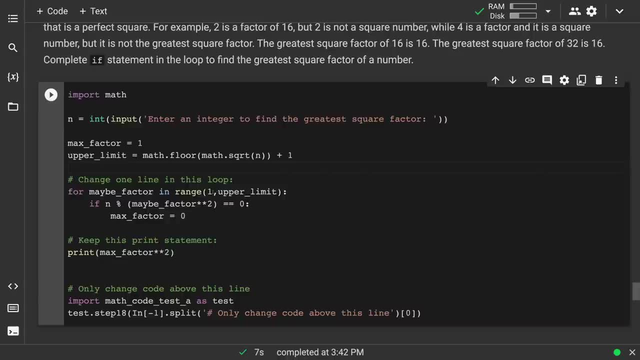 gives us the upper limit Square root of that number, and then, but we really want the next number Now, what do we have? Now, my range from one to upper limit. so, and remember this upper, that was the square fact, the square root factor. 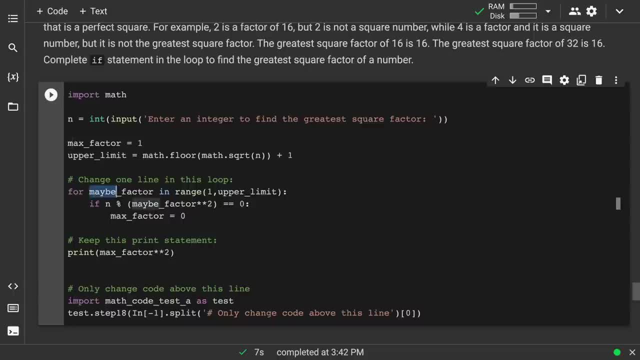 I square rooted it first, So for maybe factor in that range, so it's going to go through, and maybe factor is going to be one, and then it's going to be two, then it's going to be three, you know, up to this upper limit. 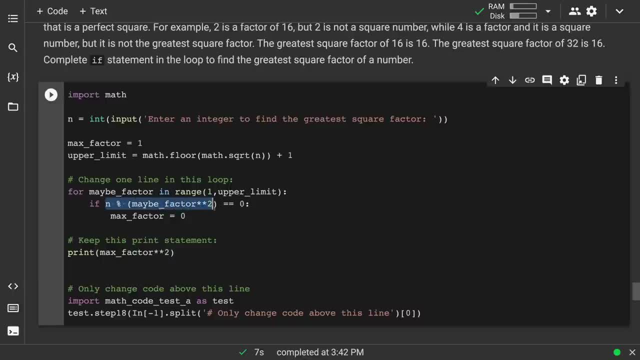 So if n modules, maybe factor squared, equals zero, So that's it, These factors, if I square them, is that a factor? Can I divide that out? And if that is, then max factor? you see, it's not going to be zero. what's it going to be? 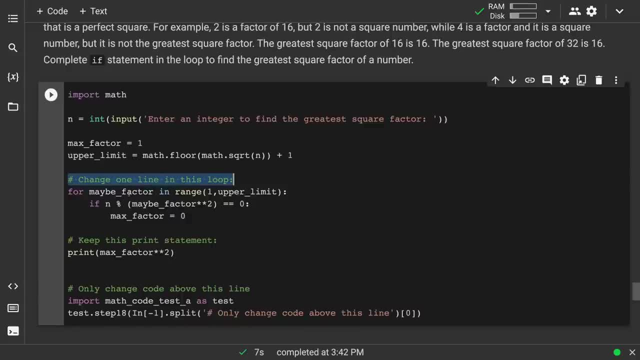 And that's the idea with some of these change one line. So if you go through and think about what you're doing, then we see, yep, I'm going through this range and maybe factor is it, and then finding square factors. 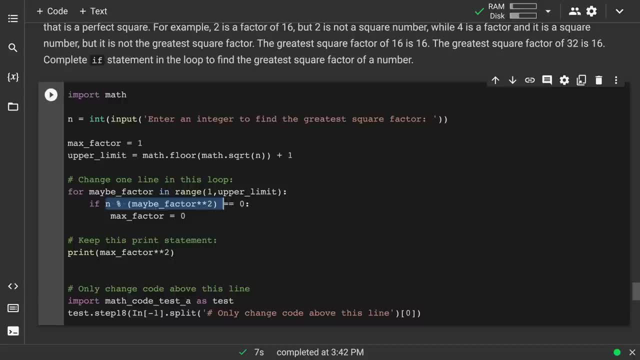 if n divided by maybe factor squared, that gives a remainder of zero, then max factor equals maybe factor. So that's what we change. There we go And again knowing that these were the square rooted. so for our purposes here we'll just print it out: squared. 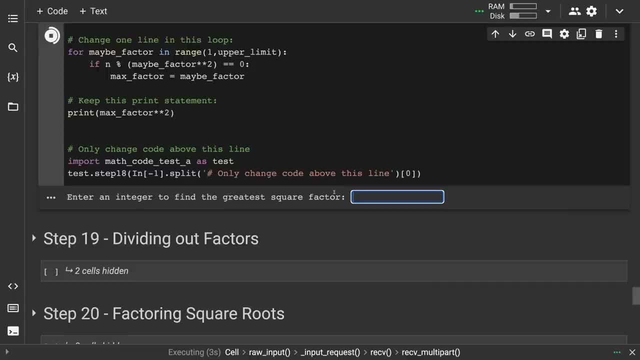 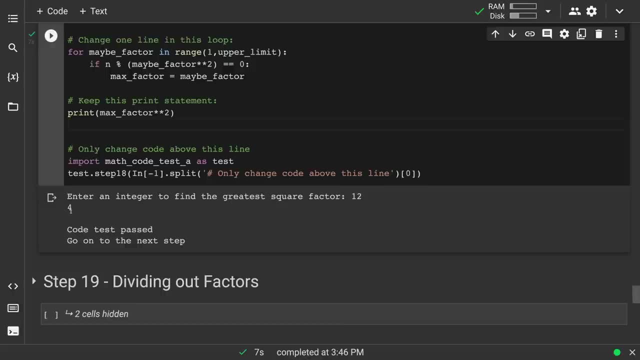 So we'll see this here. So if I have something like twelve, the greatest square factor is four, because two, you see it prints out squared two squared is four, and that's a factor of twelve. Three squared is nine does not. 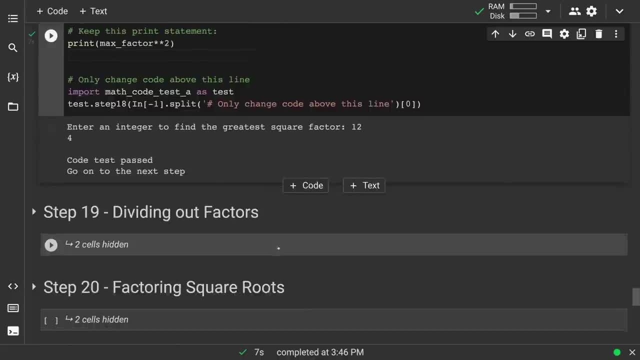 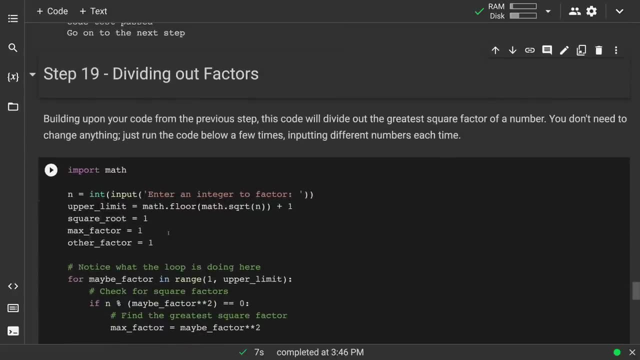 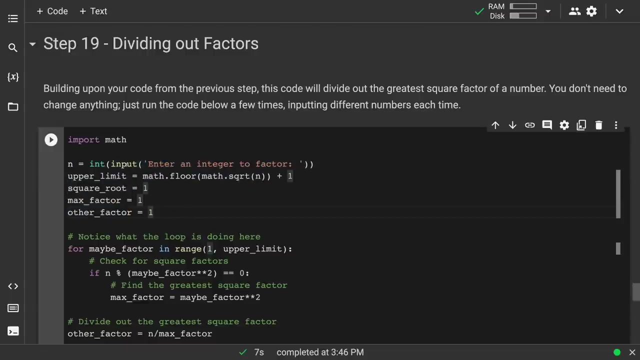 work out to be an integer, Okay. so here we're going to build upon that code and then we're going to have all of this, because when we look at factoring out square roots, that's kind of what we're building up to here. When you have a square root, 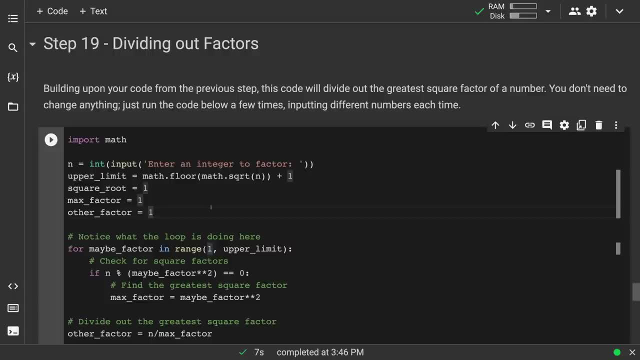 that doesn't work out perfectly, but yet you can factor it a little bit. that's what we want to do here. So I still have get the same integer, same upper limit, and I just put all these variables equal to one, because we'll change those Square root, max factor, other factor. 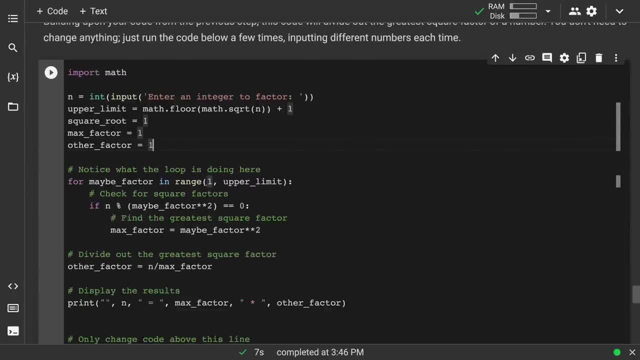 Alright, and then take a look at what this is doing. same thing, because I still got that same upper limit and so still maybe factor is going through that range. check for square factors, just like we did before, and then there we go, and in this case, max factor. 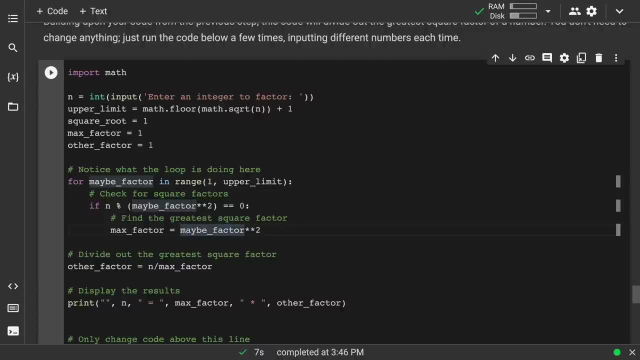 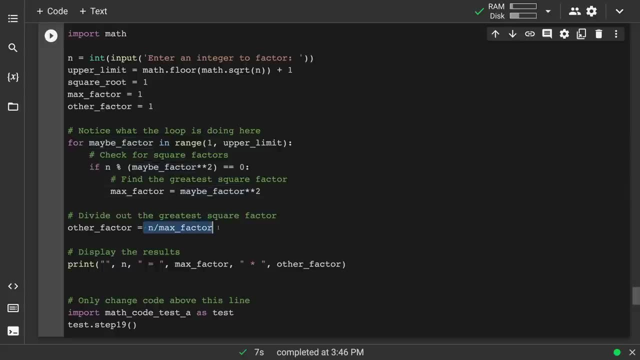 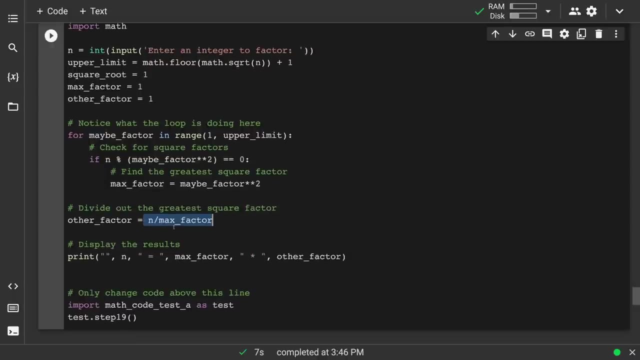 equals maybe factor squared. There we go. and then other factor is n, the original number divided by max factor. So there we go. so what we have is the result is going to be that original number n equals this times this, And we're just looking at. 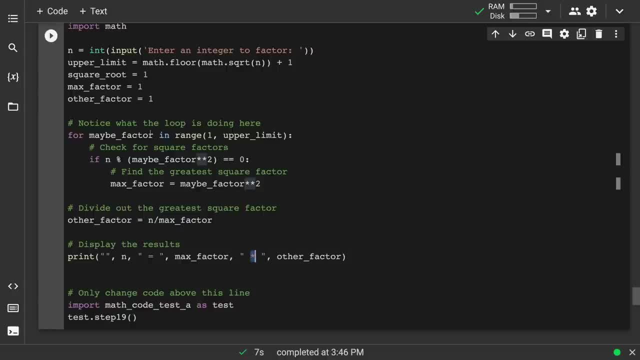 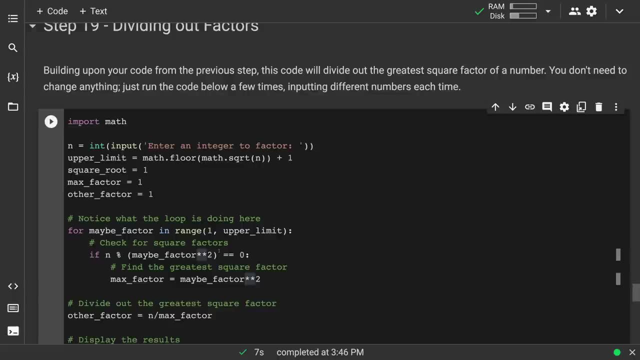 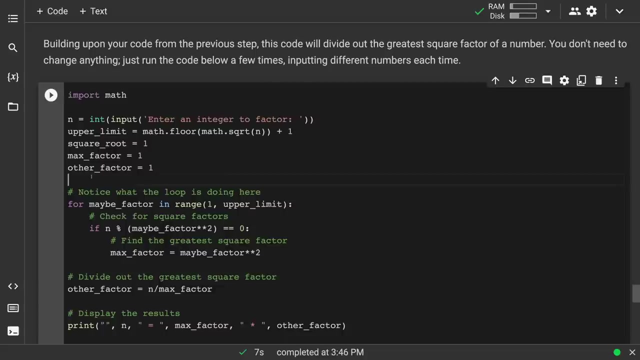 how that divides out. So in this case you don't need to change anything, because I thought that this was a little bit, you know, a little bit complex to try to follow what I was thinking through. so I didn't want to have you have to change anything and just 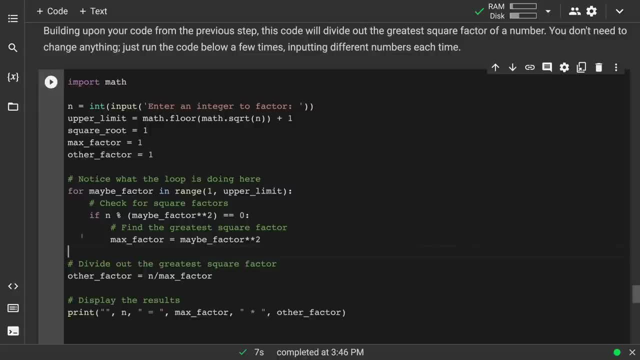 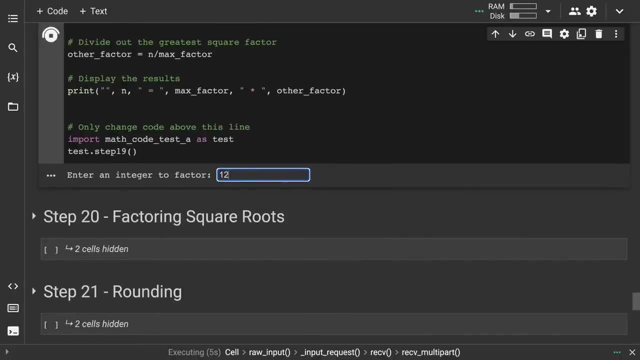 take a look at what's going on here, how we're dividing that out and then when you run it. so if I enter an integer to factor, maybe I'll do the same. 12 here- see 12- equals 4 times 3.. 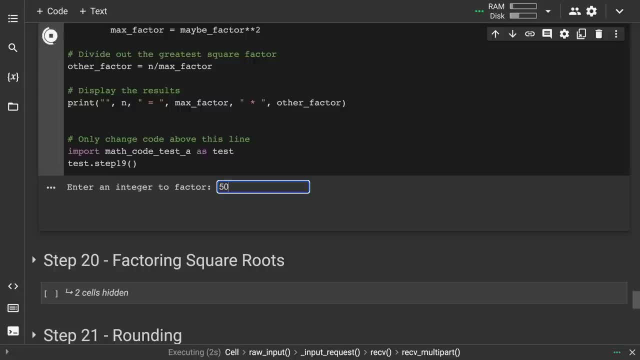 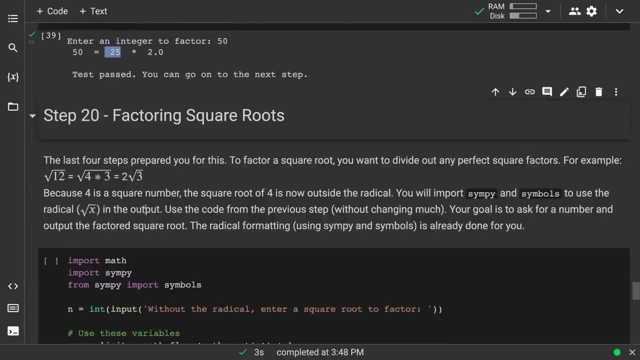 Or if I do this again, let's say 50,. 50 equals 25 times 2, and again that first part is a square factor. So now there we go. the last four steps prepares you for this. So factoring out a square root, this is kind of what we want. 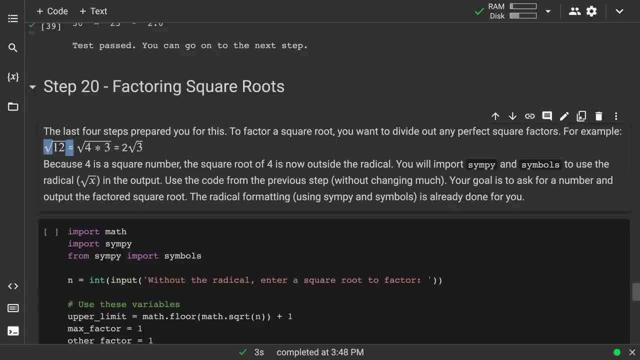 12,. if we look at the square root of 12, is 4 times 3, so then, since 4 is a perfect square, the square root of 4 comes out and it becomes 2 root 3, and that's what we're kind of building. 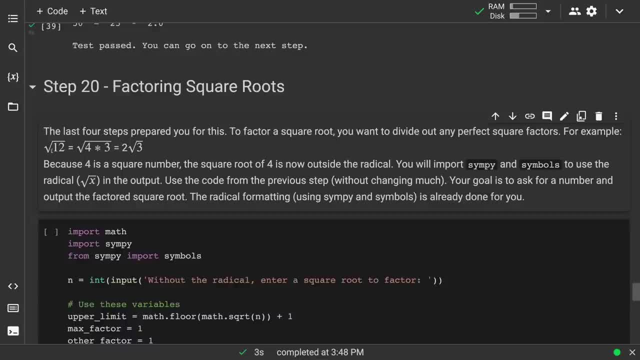 that's what we're building this code to do is this: whatever is that square root number? I'm finding the greatest square factor and then that comes out because the square root of 4 is 2,. 2 is on the outside. now. 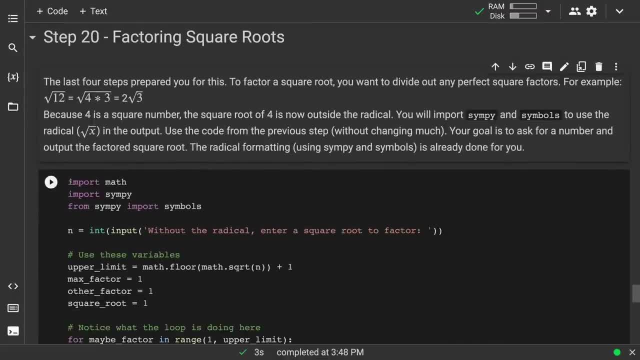 Alright, and in doing this, we're going to import math because we have square root, and for our final output, we're going to import sympy and symbols, because that's going to give us a nice output at the end. that looks like: 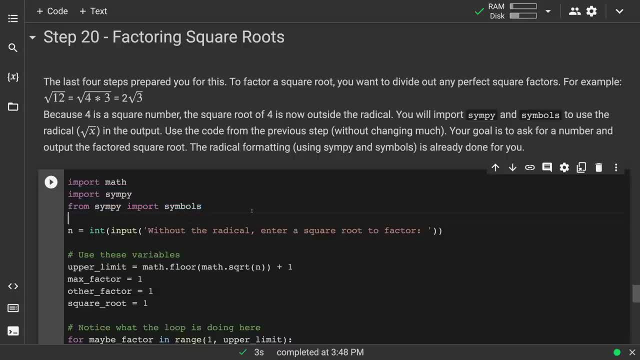 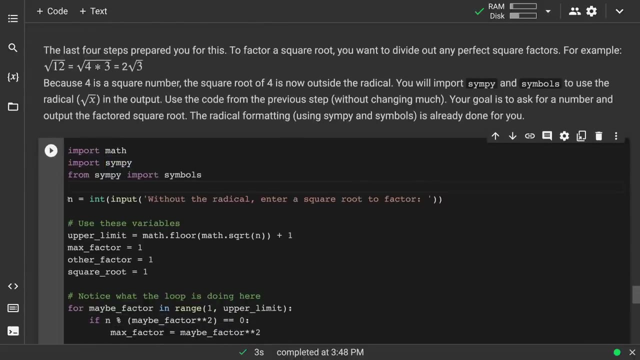 this. So that's the thing you know. Python outputs a certain way and then if I wanted to output that looks more like math symbols, that's what we have: symbolic Python Using our math symbols. So similar input without the radical enter a. 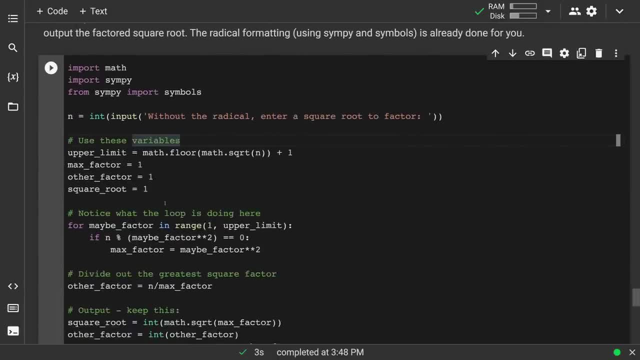 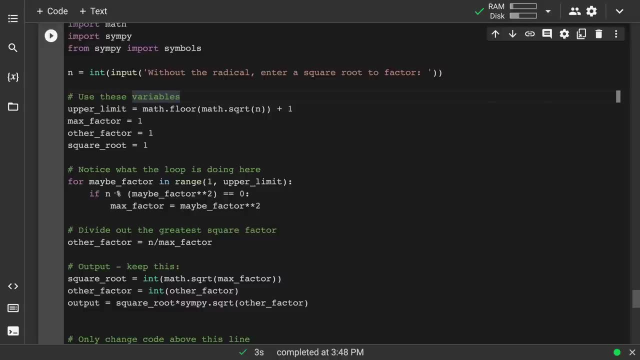 square root to factor, using those same variables, dividing these same type of thing where we're finding maybe factor and then max factor. Now, in this case I kept it like this: maybe factor squared, so the max factor squared, and then we divide. 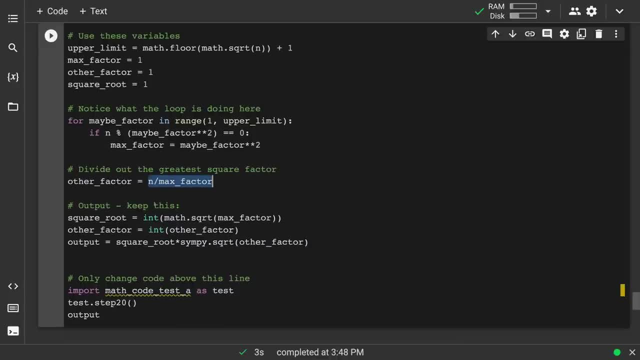 so now we do the output. so I am going to square root it again. Yes, and I realize that up here there's maybe factor squared and then down here I'm square rooting it again and the key is casting it as an integer, because this will be an integer at this point. 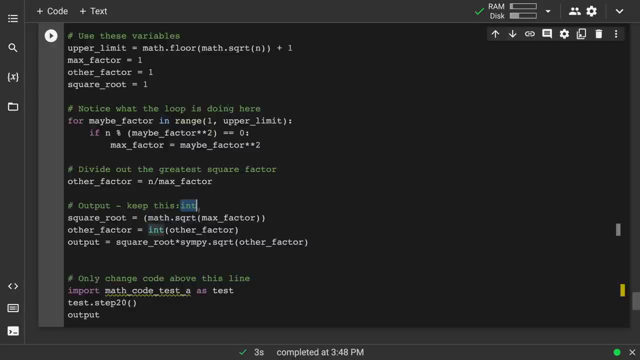 Oops, Did not want to do that. there we go, Because this will be an integer. at this point, casting it as an integer. Okay, so that's the square root. and then remember other factor: out here was my original divided by that max. 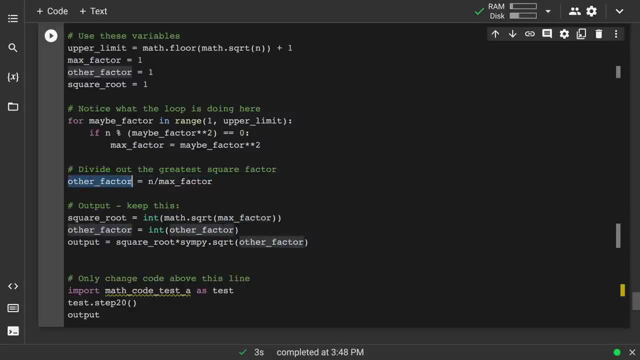 factor and if there's anything left over, that's this other factor Down here. I'm casting that as an integer and you know, that's it. I'm just taking this other factor, but casting it as an integer. 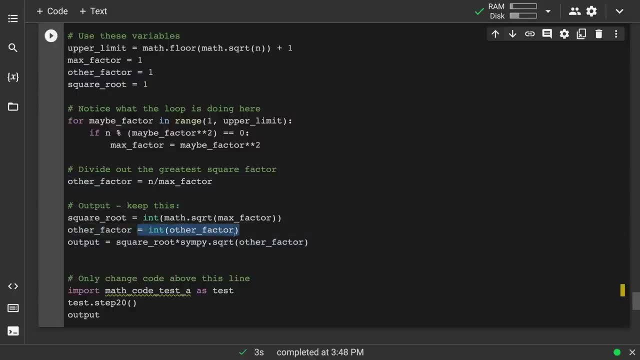 And you see that you can do that with variables. So now it's an integer and now the output is square root, which was this variable up here: times sympy. so this sympysquare root is different than mathsquare root and 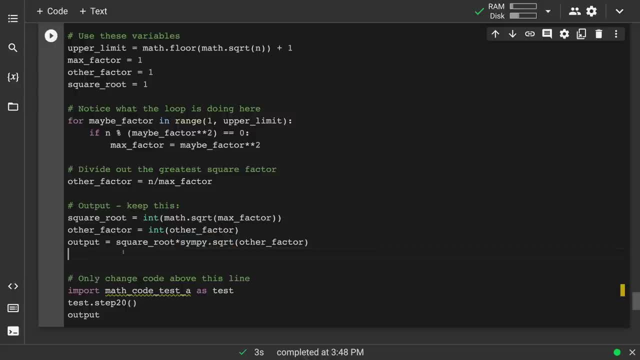 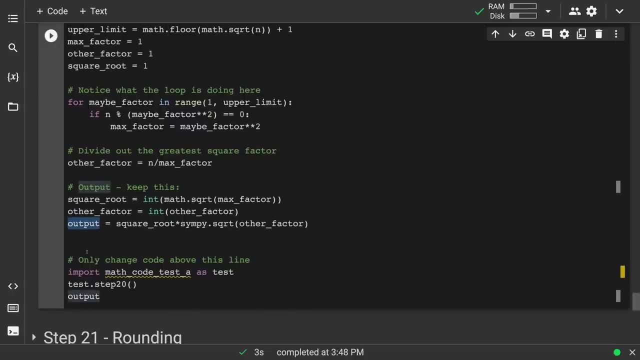 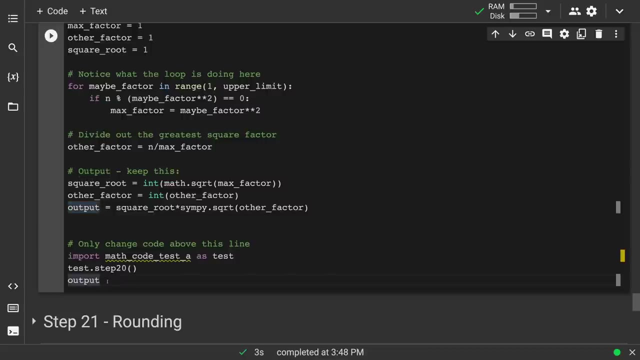 using this sympy output. I want that to be my last. I want that to be my last thing. is this output so down here after it does this for the test? that's why the word output shows up here. We store it as this here. but notice, it's not a print statement, it just says: 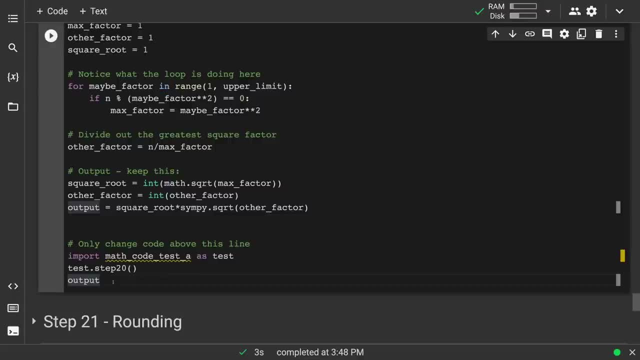 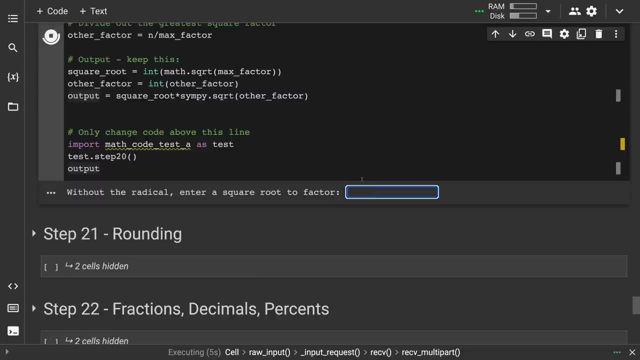 output and the last thing just says output and it will display it. So these types of sympy displays. sometimes you just need to put that there: Output as the last thing, Okay, so what do we have? Let's take a look at our. 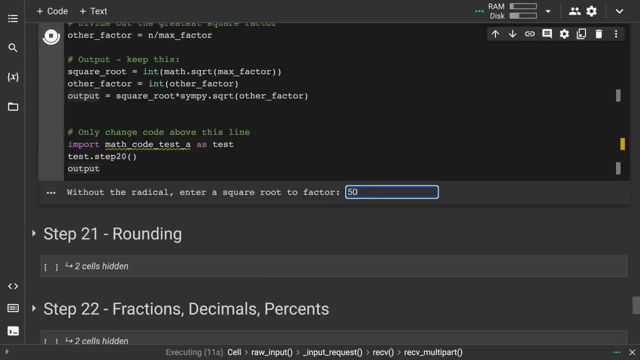 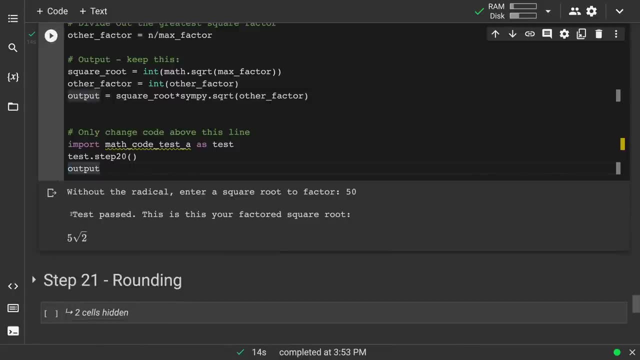 let's take a look at 50, as we were talking about before. So, and just because this came first, that's why it says test passed here, and then we see the output. but 50 factors out to 5, root 2.. 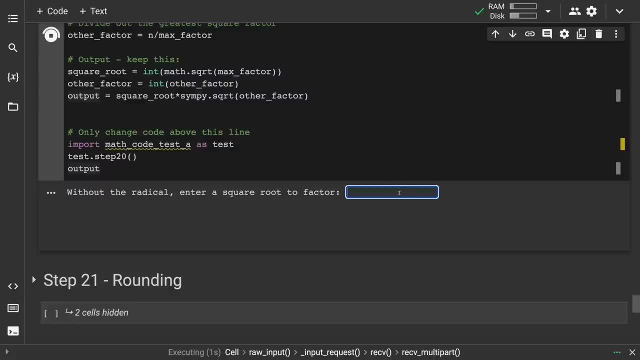 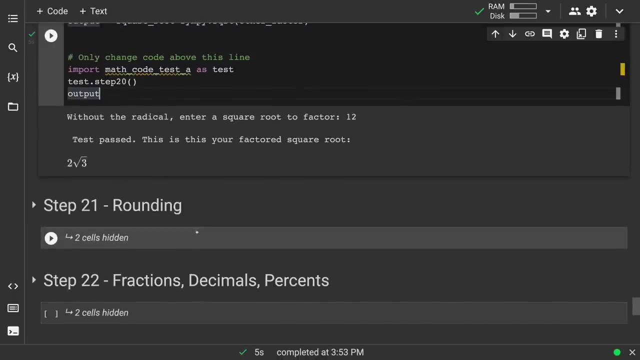 And if we run it again, then we have, you know, go back to our 12,- 12 is 2 root 3, and we can see how we can factor out these square roots. So there we go. this is now one of the things that you. 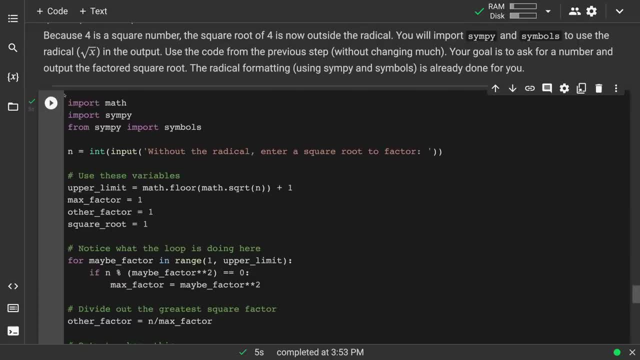 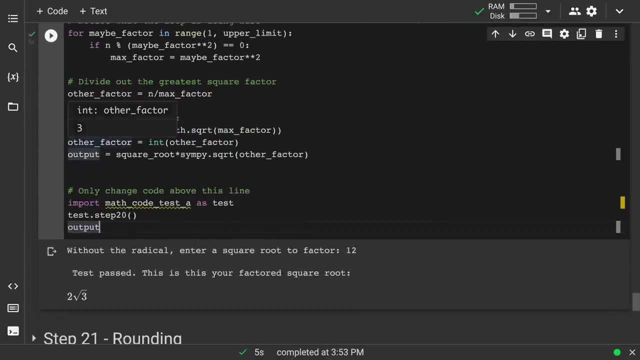 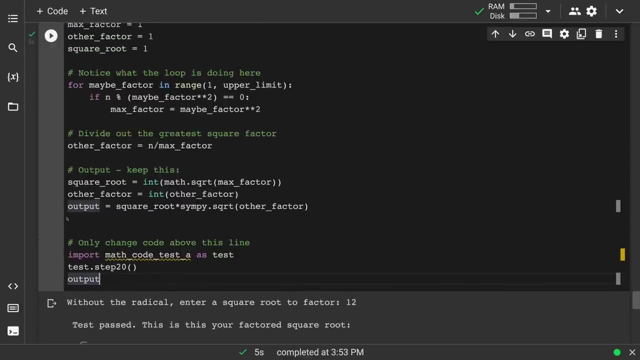 can do, and this would be a bonus. we could do this later is? we already talked about functions. you could put all of this in a function. You know all you know. you don't need the testing part, but the output. you could put this all in a function. 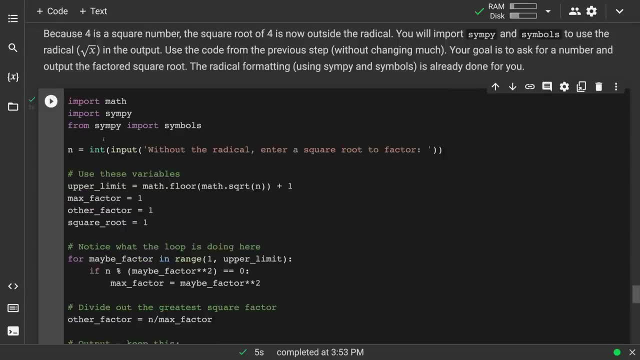 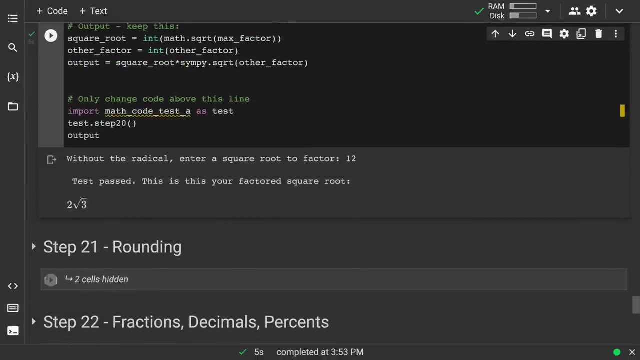 that would factor square roots for you. So, just like you have mathsquaresqrt to output the number, which may be a decimal, you could actually make your own function that would do all of this and then output a radical, You know, like this. So some interesting. 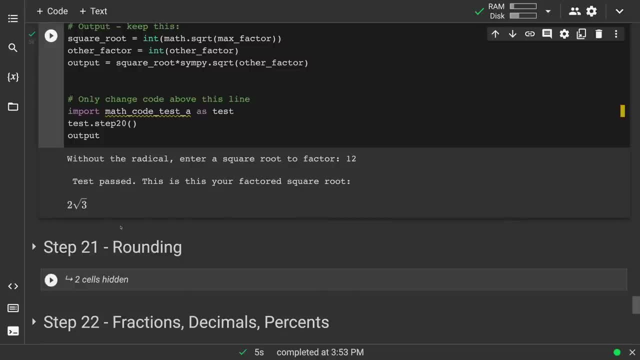 things that you can do, And that's kind of I wanted you to see the buildup of this and how we can use these- you know, loops and factors- and do this to factoring a square root, which is something that's. 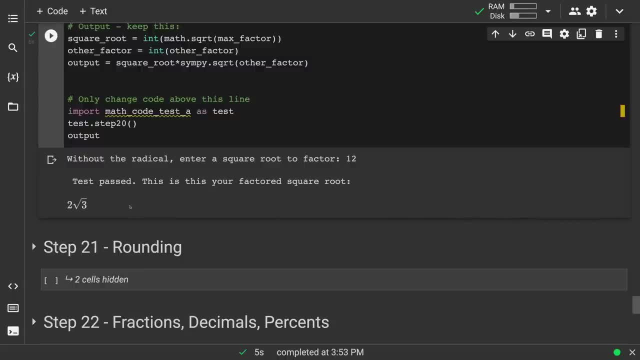 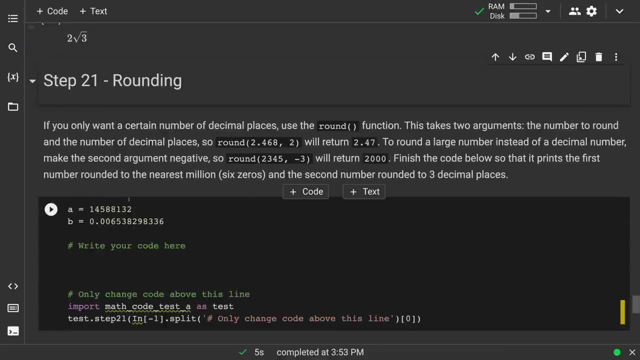 you know, pretty interesting in math, useful for some math you get into and that you can write code to do it. Alright, here's some rounding, just interesting things. So if I just say round, it'll round it to a whole. 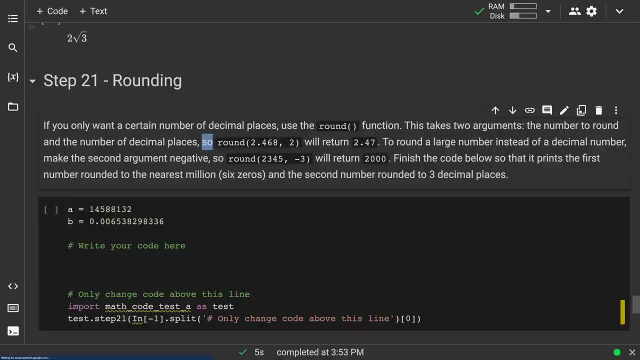 number. If I have something like this: if I round comma and then have a number that'll tell me how many decimal places, and if I have this round and it's a negative number, that'll be for big numbers. so 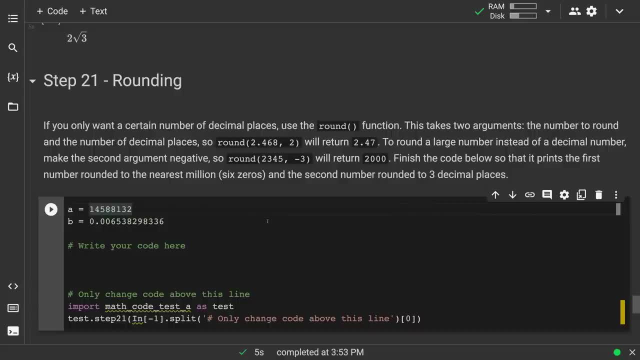 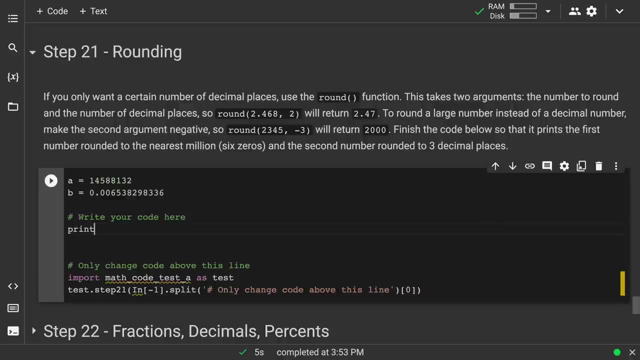 it'll give me that many zeros. So there we go. So, first number rounded to the millions. the second number rounded to the six decimal places. So, and I do need to go back to my print statements, print round. and the first number: 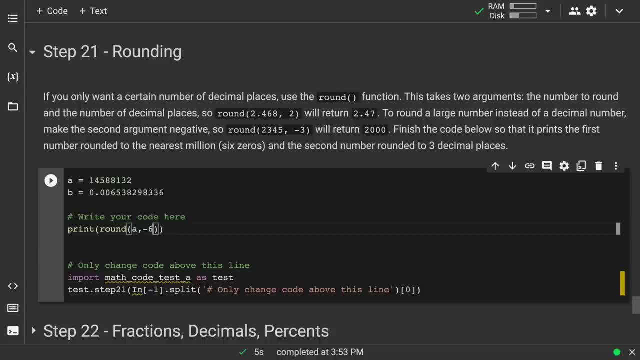 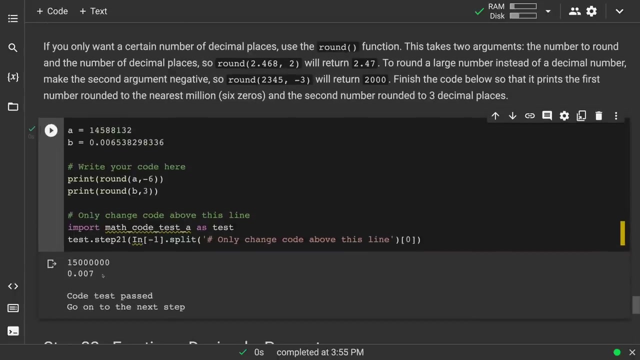 six zeros, so I have to make it negative six And then the second one print round B, and I wanted three decimal places, so it'd be three. There we go And we can print. So there's my six decimal places. 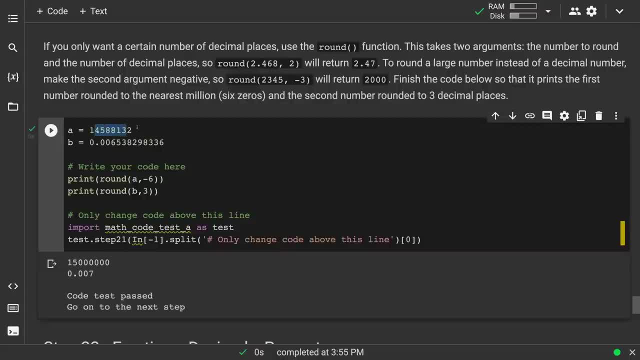 and you see, then you know, I don't want it to round to the next integer- it already is an integer- but I want fourteen million, five hundred thousand rounds to fifteen million, And then the next one, yep, rounds to double, oh, seven, of course. 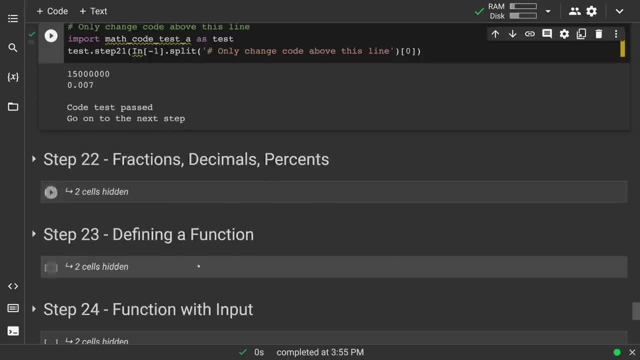 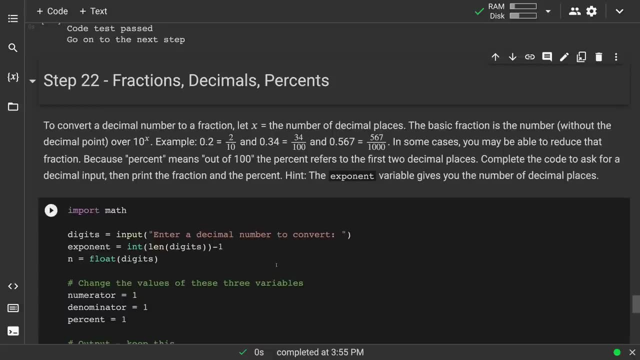 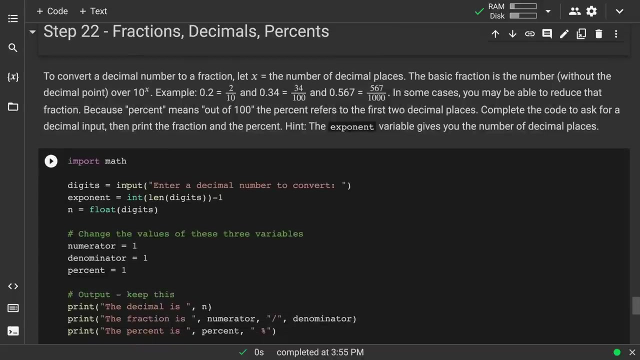 Alright, There we go And fractions, decimals and percents. So we could see here- and we've done some things like this before- that here we're going to take the input as a string. see, I'm going to import math for later. 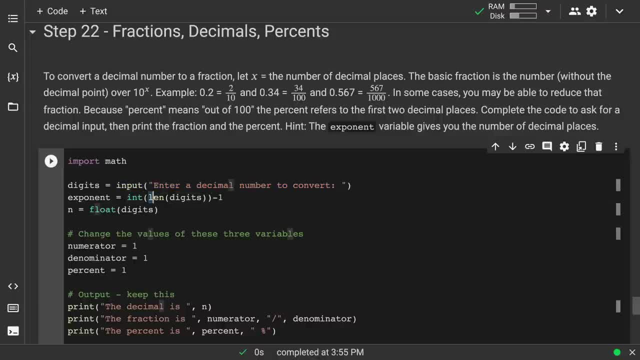 take the input as a string and as a string. every string has this built in L-E-N, which is the length of that string. So I want to take the length of that string and then I need to cast it as an integer. 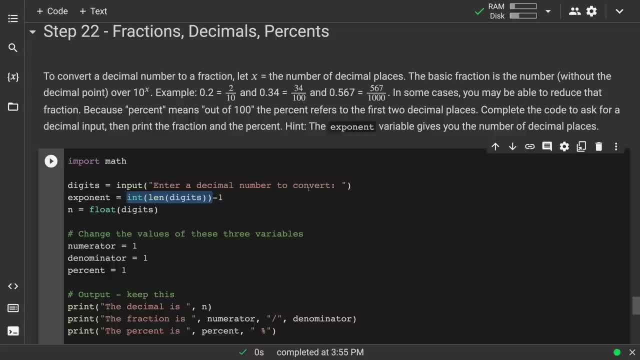 Now remember, the person who enters this in is going to put a decimal place. so that's why I have to subtract one, because I don't want that decimal place. I just want how many decimal places without that dot, Alright. so that's going to be the end. 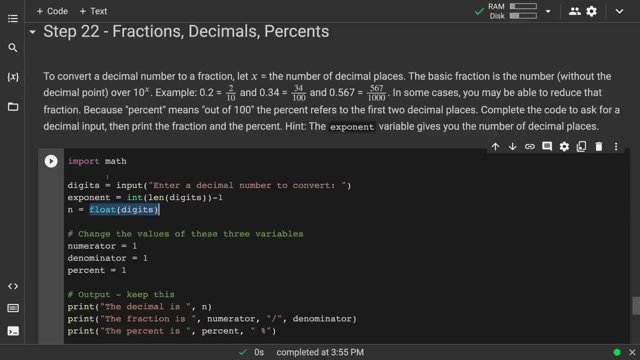 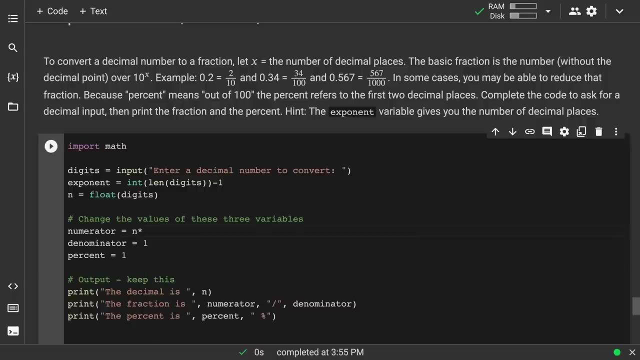 So I'm going to take the exponent and then, now that I've done that, now my input digits, I'm going to cast that as a float, So the numerator is going to be N times 10 to that exponent and then my numerator is actually going to be an integer. 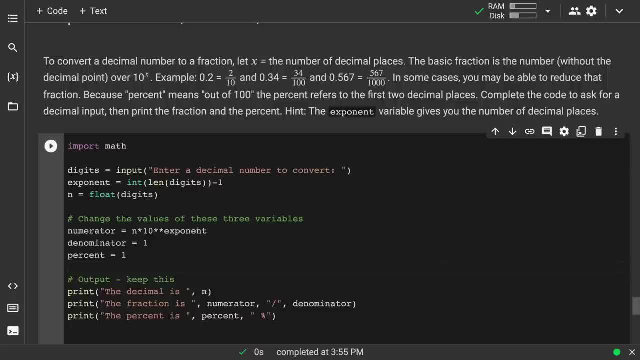 So anything with three decimal places. it's going to be times 10 to the third, And doing that is going to move the decimal place over, and then my numerator is actually going to be an integer And the denominator is that: 10 to the third, oh, 10 to the. 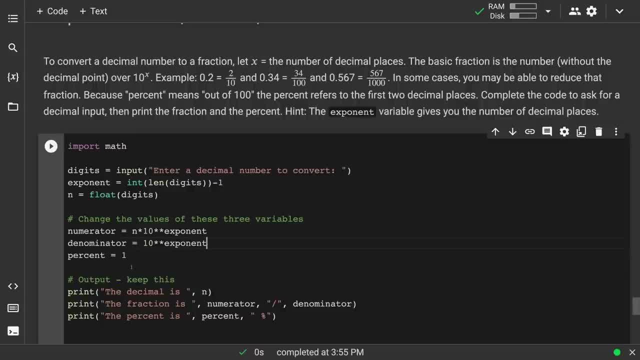 exponent. There we go. so there's my fraction, And this is really what we're doing. anytime we're converting fractions, but now we're just writing code to make it easier. So how many decimal places? That's really what this is essentially doing here. 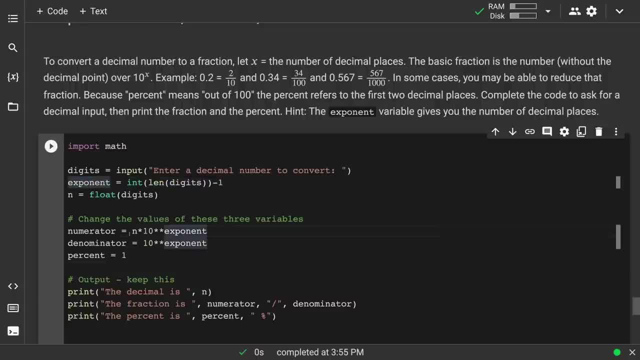 How many decimal places am I talking about? And then that number times 10 to that, those decimal places 10 to that exponent, and the denominator is 10 to that exponent. So then the percent, because now that I have it as, 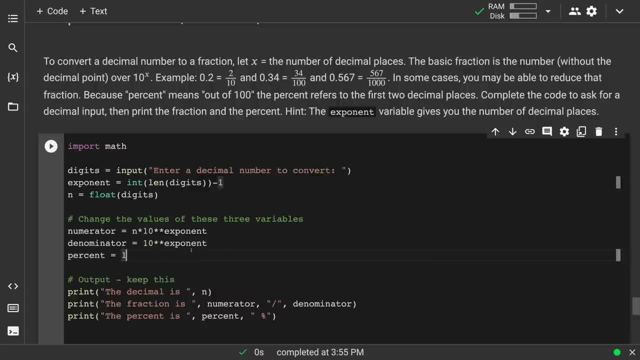 numerator to denominator. Now I actually really can just go back to n if I want, or I could put numerator divided by denominator, whichever one. But I could do n times 100, which it's always times 100, because it moves the decimal place over. 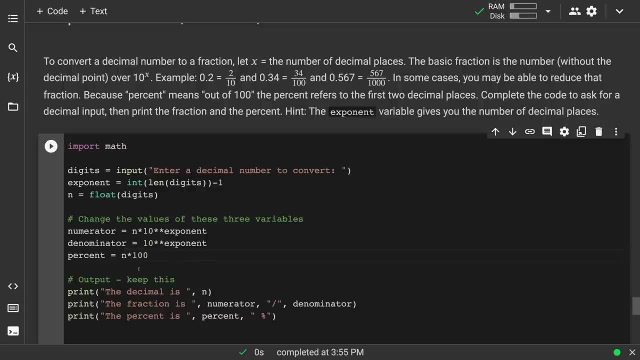 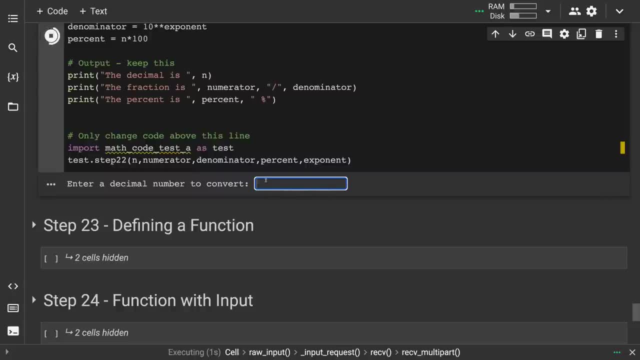 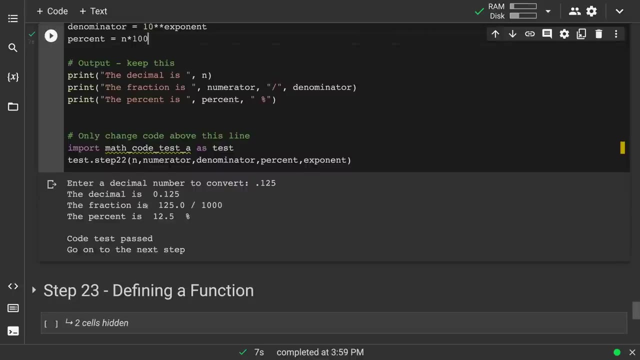 And so that's it. The first two digits are your percent, so n times 100.. 100 gives you the percent And we can run it. So if I have somebody enters in something like 0.125, there we go. 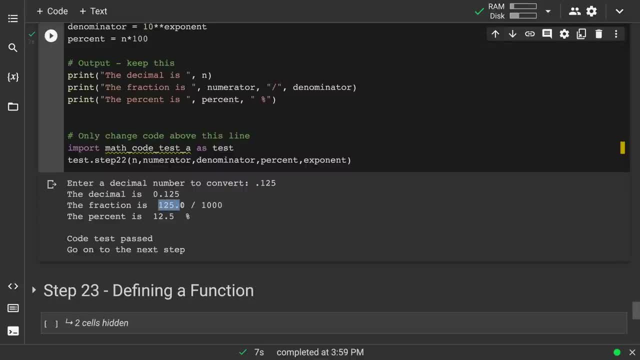 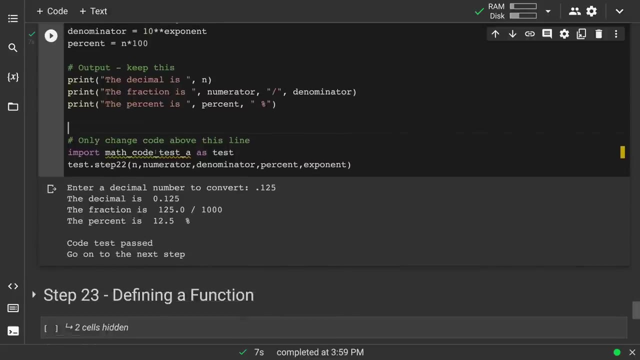 So the decimal is 0.125.. The fraction is 1.25 out of over 1,000.. And the percent is 12.5%. So there we go, Converting And you enter Input: fraction, decimal, percent. 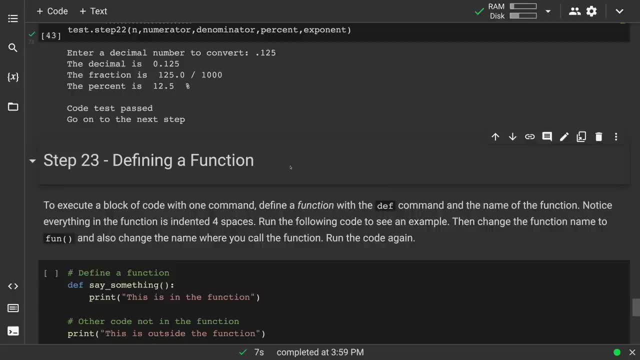 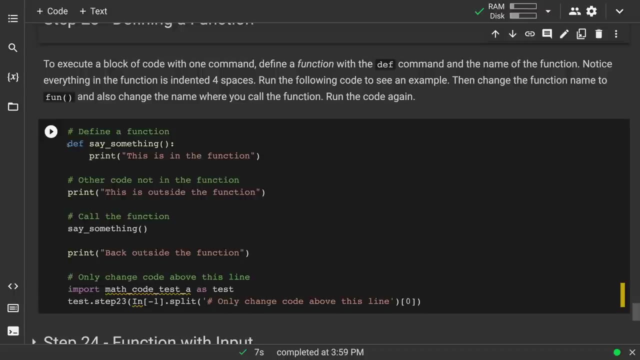 And this is where I was saying that you could define a function here where you can execute a block of code with one command. So here's the function definition- DEF- and then the name of the function: Open and close parentheses. that may take input, but they don't have to. 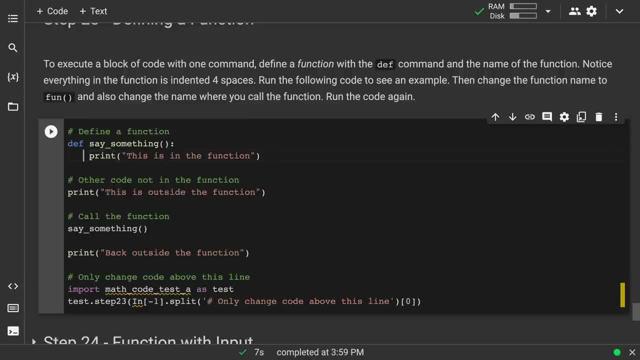 And then input, indented four spaces: 1,, 2,, 3, 4.. So DEF: name of the function, colon: Anything in the function. it can be as many lines as you want and it can have comments. 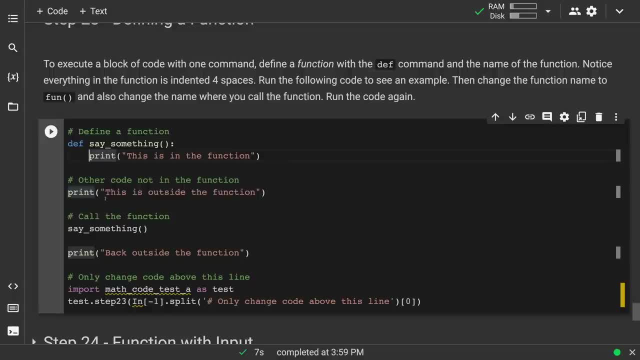 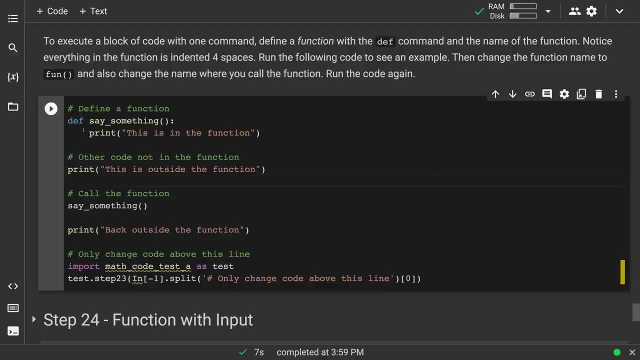 Just indented four spaces And then there you go, Here's something outside the function, And then that function is defined And then it's then called. It won't do anything until it's called here. So I could have this function definition. 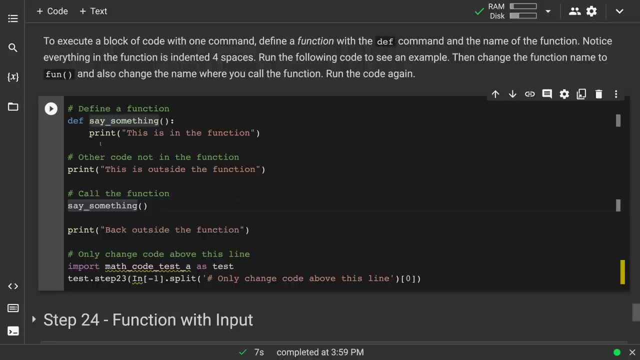 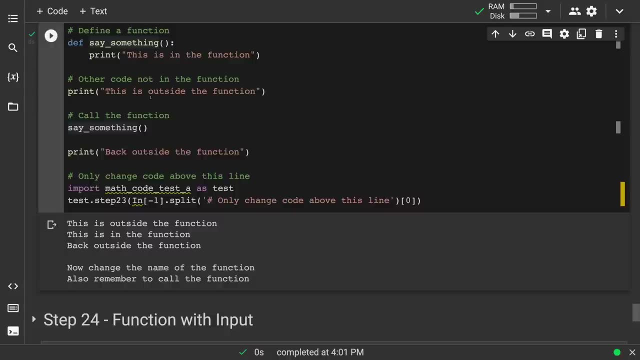 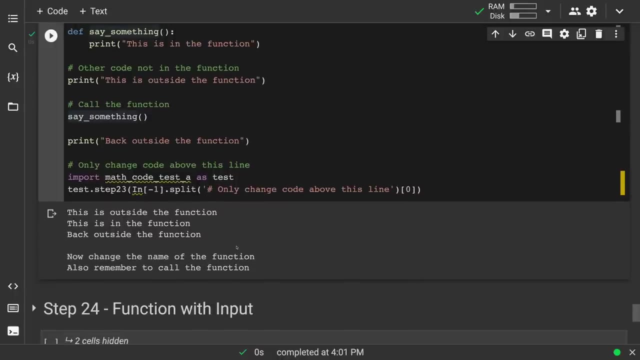 And if I took out this line it wouldn't do anything. So now it'll have this is outside the function, Then it'll print This is in the function and then back outside the function. There you go. Now change the name and remember to call it. 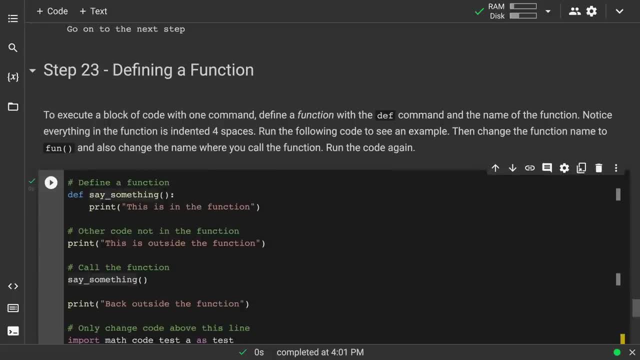 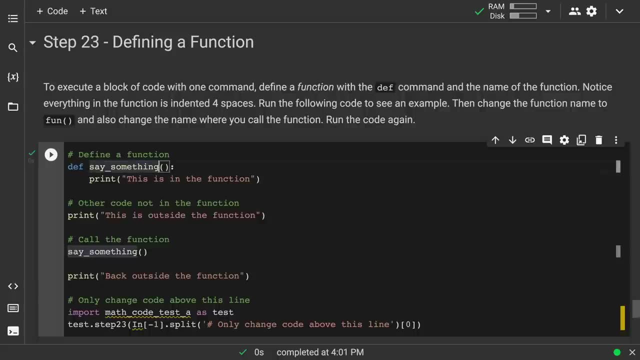 So there we go, And then we want to run it, then change the name to fun, Because can't spell function without fun. So if I just change the name, I'm going to call it fun, And now I'm going to call the function. 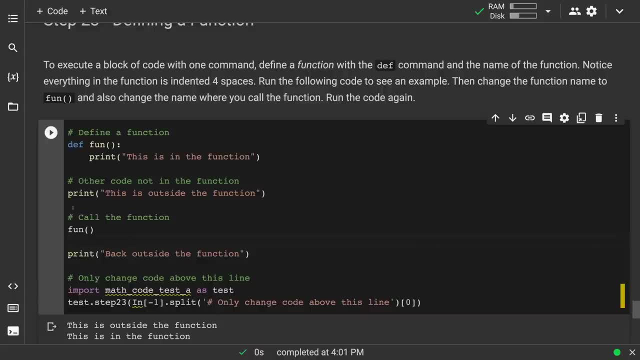 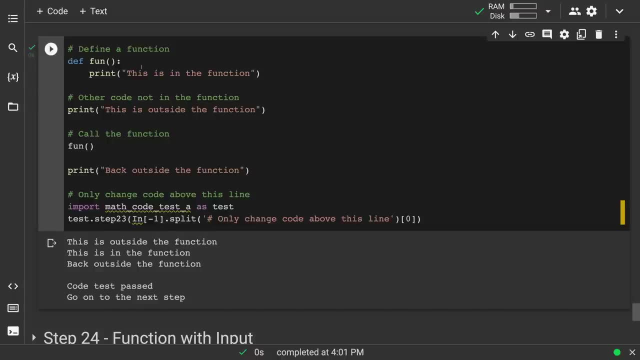 So that's what is the function. call is when I, you know, when I tell: all right, let's run that function. Now there you go. Same thing to show you how to define a function and then call the function. And then here's one with input. 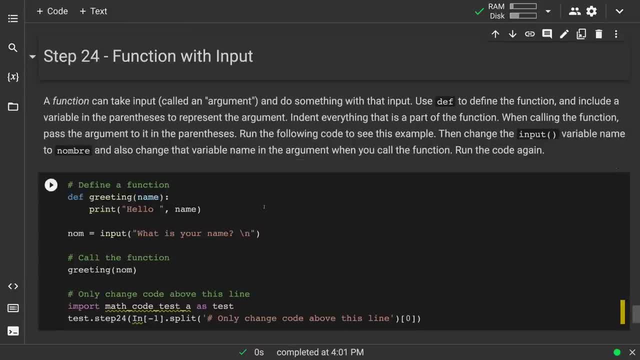 So it can take input, any input. We're going to call an argument. So there you go. Now, right here, it's telling me that it's, you know, called a function called greeting. It's going to take this input which will stores variable name. that's within the function here. 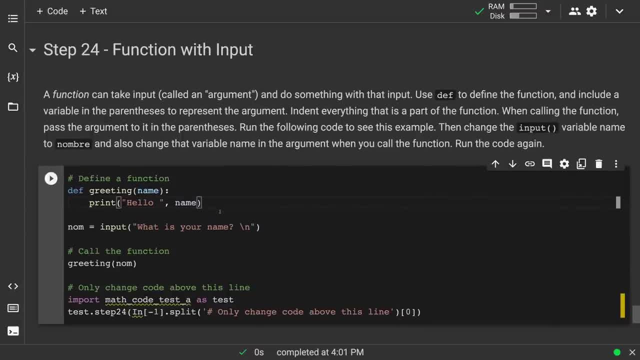 and it's going to print hello, whatever the name is, now here outside the function. So notice at the end of your function: skip a line, at least one line. So then that's the break. And now this is definitely not in the function. 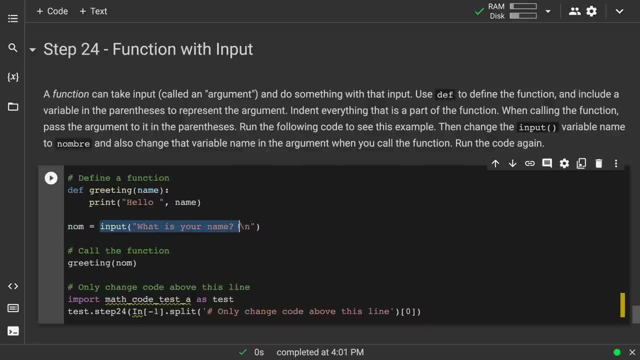 And then the input and casting it as a string, which is: it is a string and we'll keep it that way. What is your name? And notice inside the quotes that slash n will indicate a new line. So now when we run the greeting, you see it's passed. you know, I take that variable and I'm going to pass that into the function. 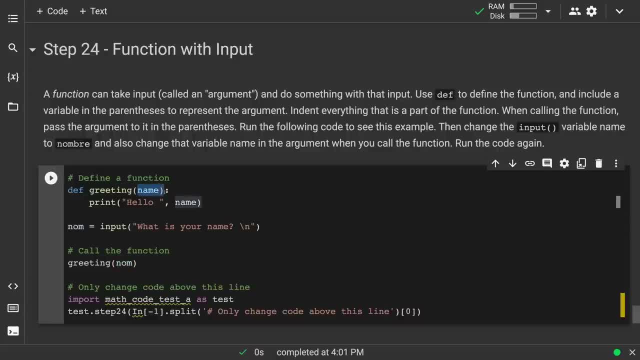 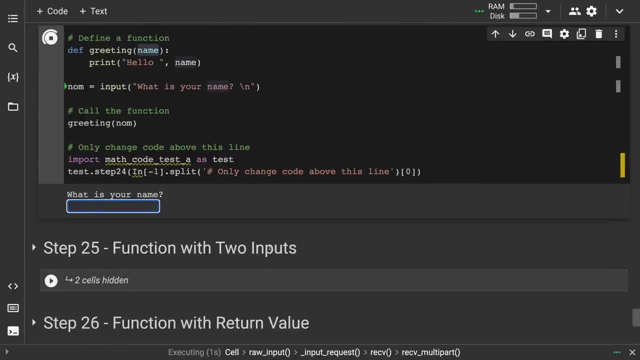 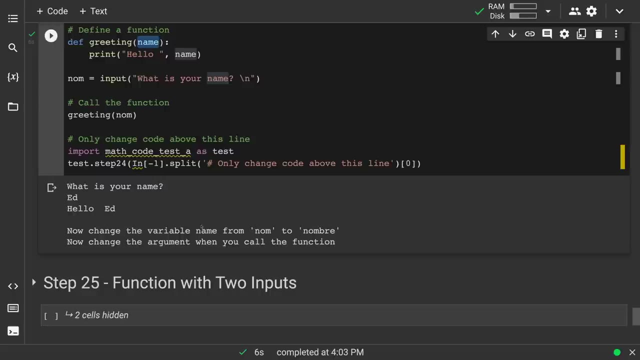 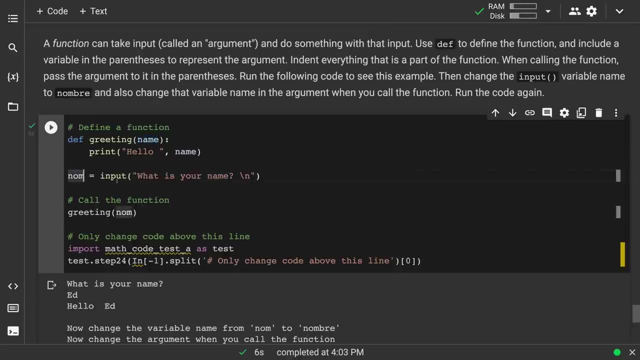 So now that Function takes input, and then it's going to be this variable and it'll do the greeting. So Here you go. What is your name? Ed Love it? There we go. And now, now that you see this working- this is just changing the this, because it's like remembering where these are- 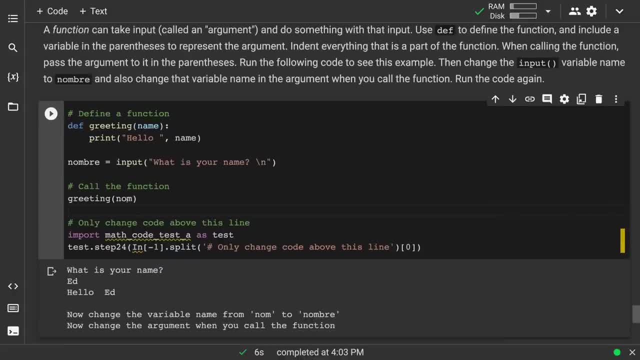 So Okay, Okay, So you know greeting, And then, when we call it, I'm going to change this variable here. There we go, So we see you know where these variables are, especially in a small, simple function like this. 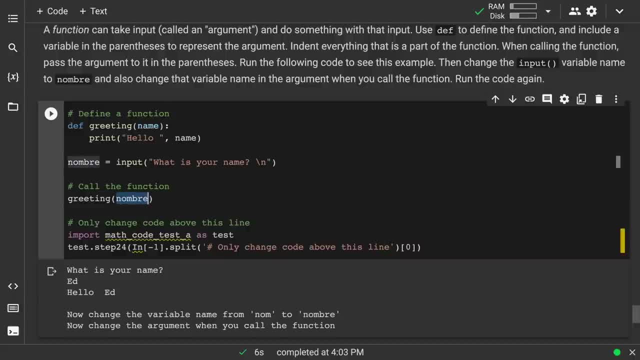 So then do we see you know this variable? how do how do I pass it to the function as an argument there, And then in the function definition it's expecting input and doing something with it. But the function of this should actually be the same. 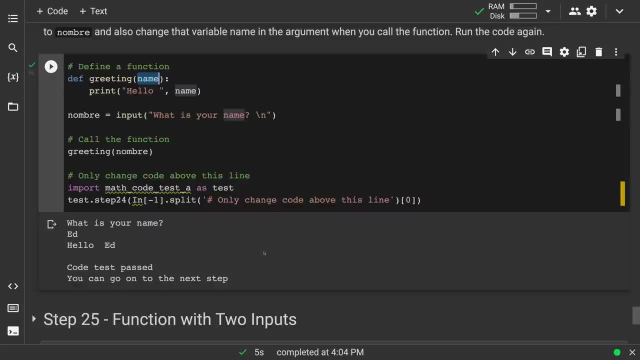 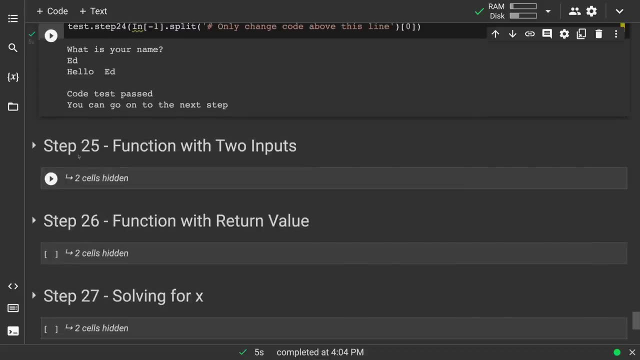 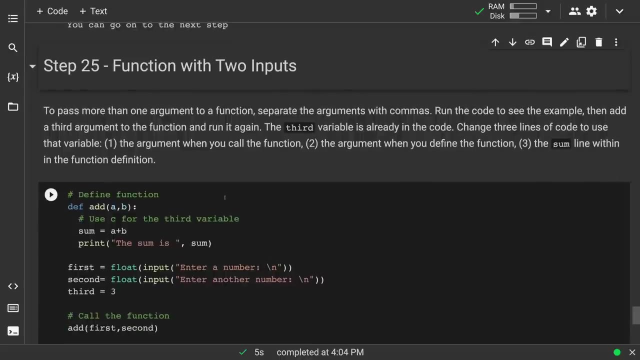 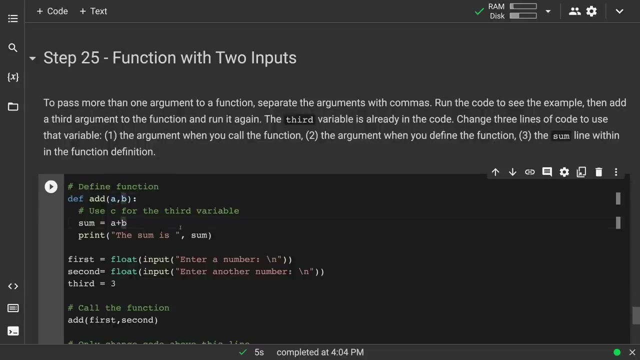 Go, Yep, See All good And these functions- which is kind of cool- You could have more than one input. So we have this, So I can have multiple input in this function And then, In this case, you know, do something with it. 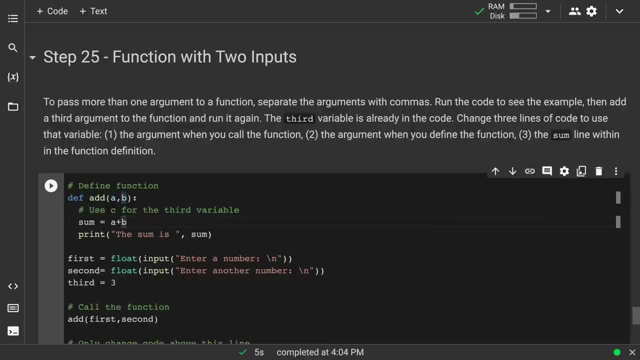 Well, we're just going to add them all, but you, you could use this for any formula you have. You see, like I just made this ad, but you can use this for whatever formula you have. make a function out of it. 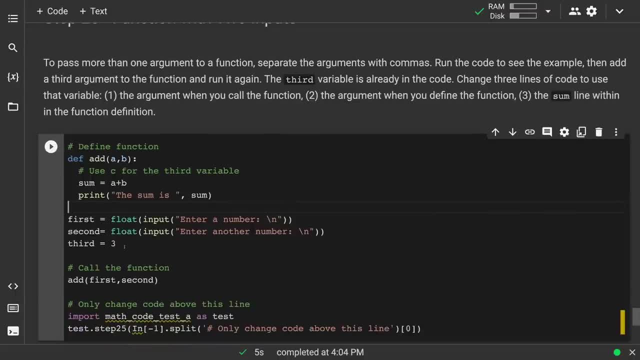 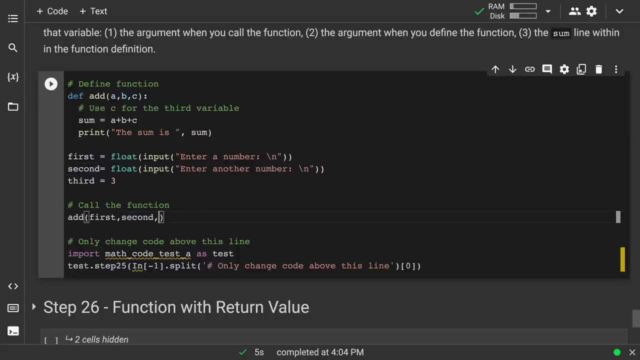 So notice here, You know the third I'll, I'll leave this as three, And then it's going to expect three inputs: ABC, And then a plus B plus C, And now down here I have to call it with all three variables. 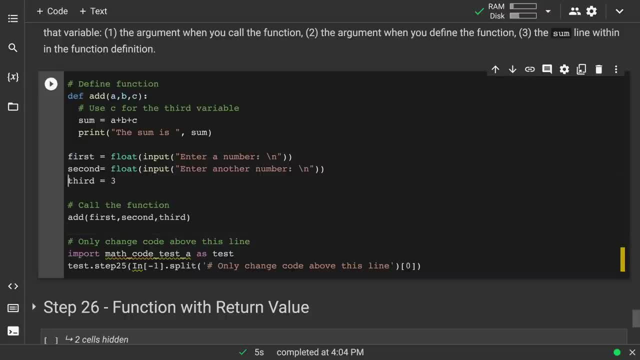 So now notice, this variable existed before, but then it just stayed there, floating, not doing anything, And then we have here. you know, now that we have have this, I'm going to call the function with all three inputs, because the function is expecting three inputs. 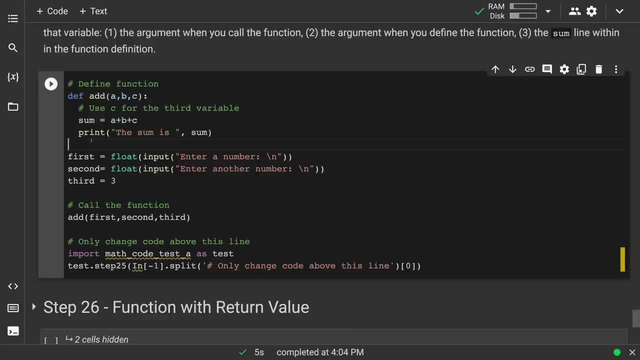 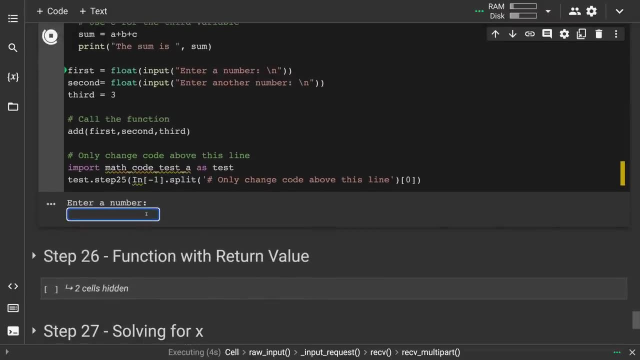 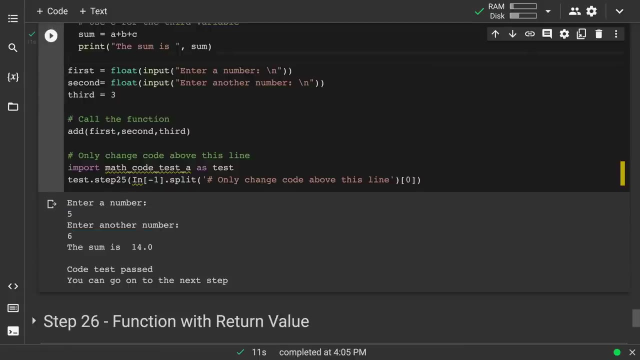 And then it's going to do something with those. And so there we go. So we see, enter a number, and I'll enter a number, and another number, six, another number, seven. Oh, because there you go. Five and six is 11 plus three is 14.. 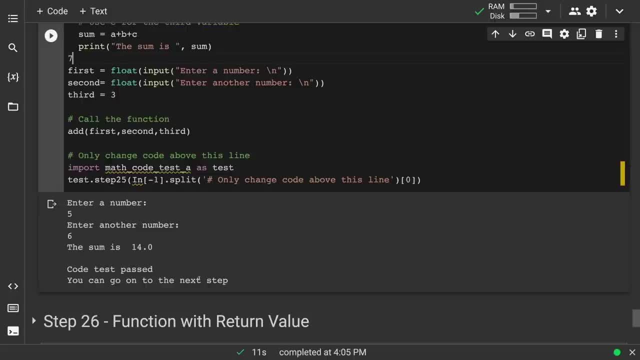 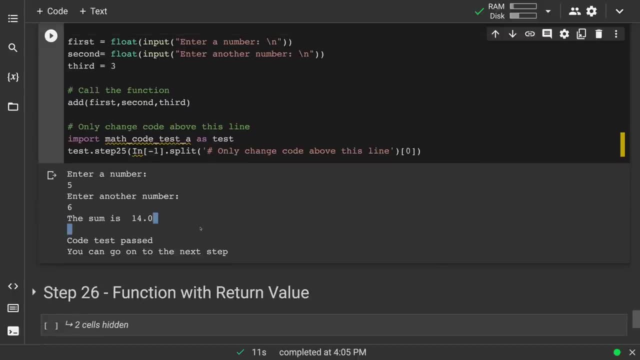 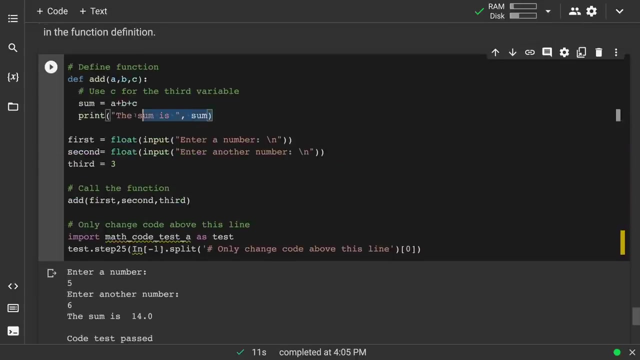 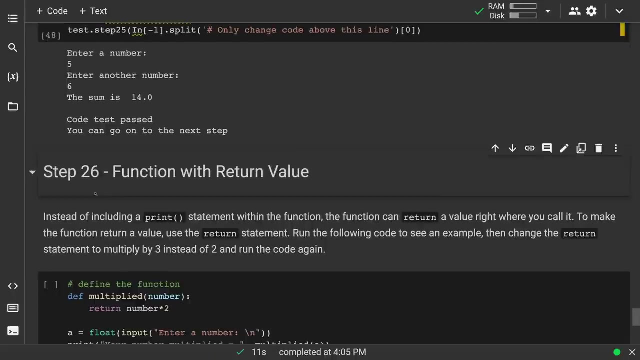 So there we go. Hey, fun with functions. Now, all the this function and the ones we had so far. they included a print statement as a way to show output, and that's good, but we could also have a function with a return value. 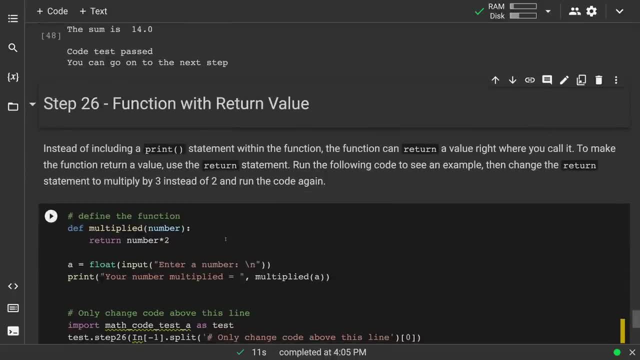 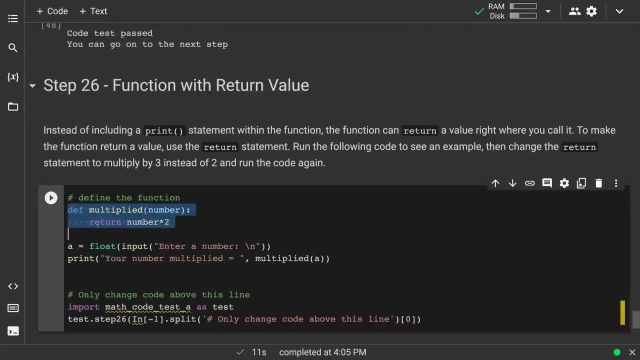 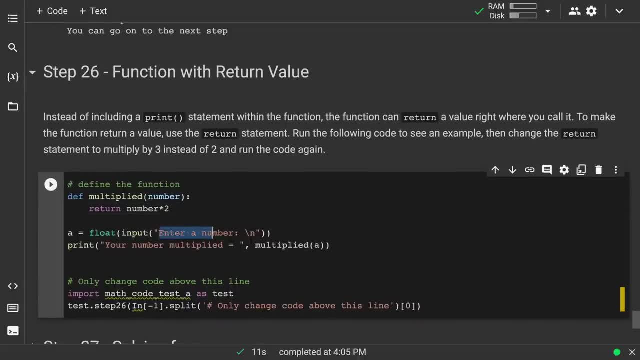 If We're going to take this, enter a number. you know there's our input, It's the float, I don't know. Store it as variable a. So now What I print Is your number multiplied equals. and then, right here, it's going to be that function. 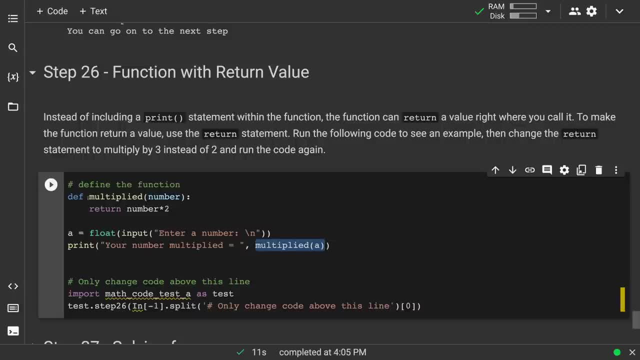 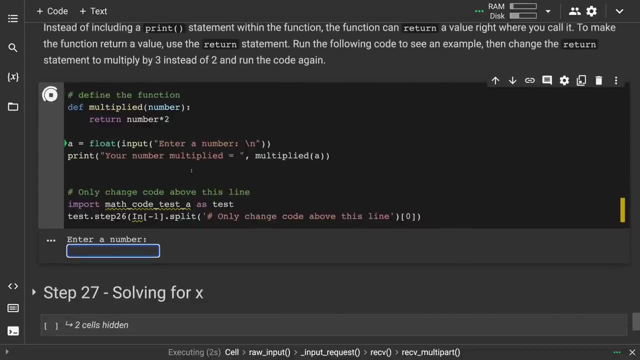 I call that function with a variable a, and that's what this is, and it's just going to take it times two. There we go, All right, So notice some of these. you run it and then we're going to change something and then run it again. 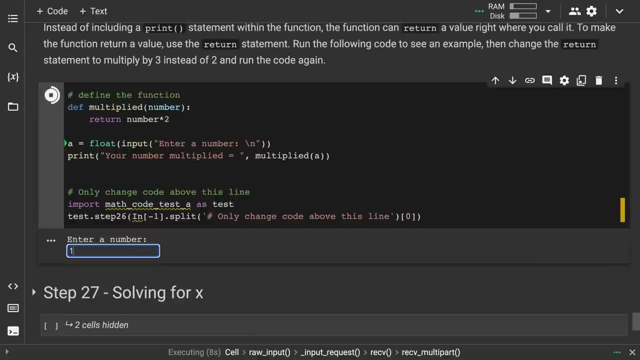 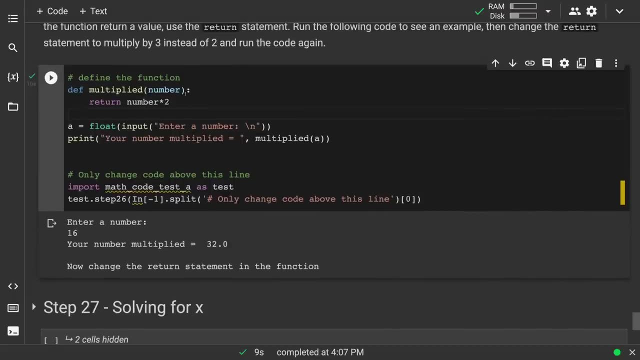 So enter a number. All right, There you go: 16.. Your number multiplied is 32.. So All we're doing here is changing the return statement. Multiply it by three instead. Everything else We actually can keep the same. 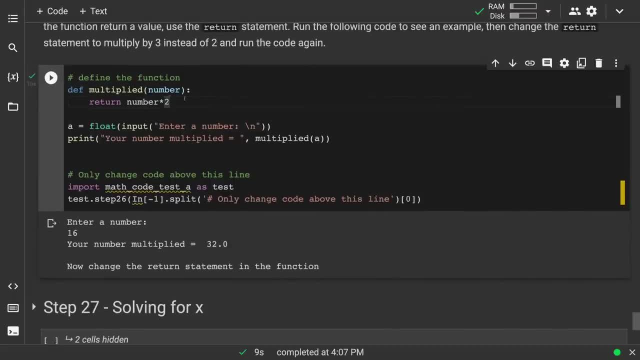 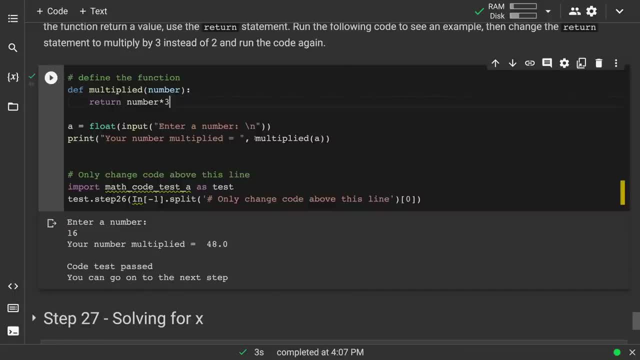 Is The return statement Is. Is The return statement is right where you call the function, That's where the number shows up. Your number multiply equals And then returns that. So that's pretty useful sometimes because we want that to just be where. 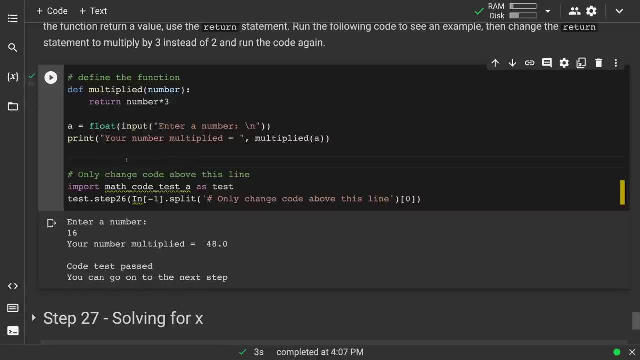 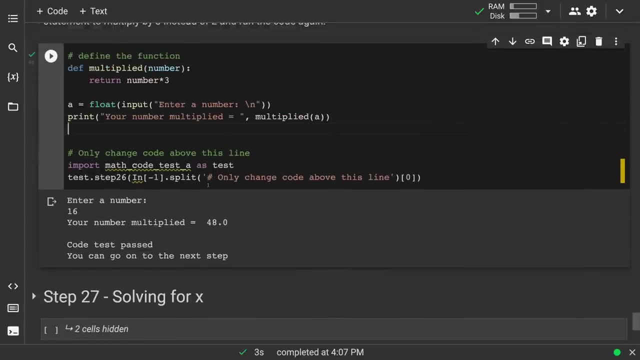 Where do I want this output to be? Right there, And so we put the function call there. So that's the return statements. Good, useful Statement here. So we have all these different things, We have all these functions. We know we're looking at factoring. 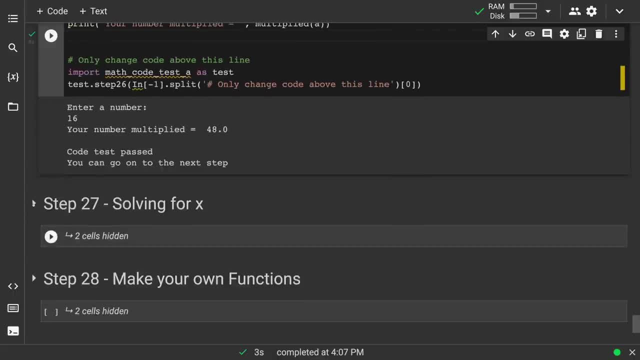 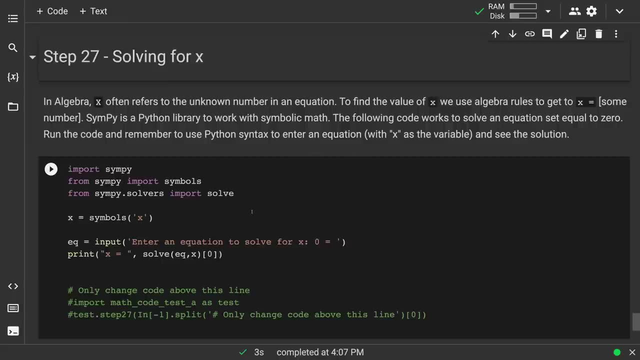 looking at solving some things. You can even just solve for x. And there you go: x as the classic unknown. Now notice, here we're importing SymPy again for our symbolic math, And we're going to take it even further: from SymPy we're going to import symbols, And from SymPy solvers we're 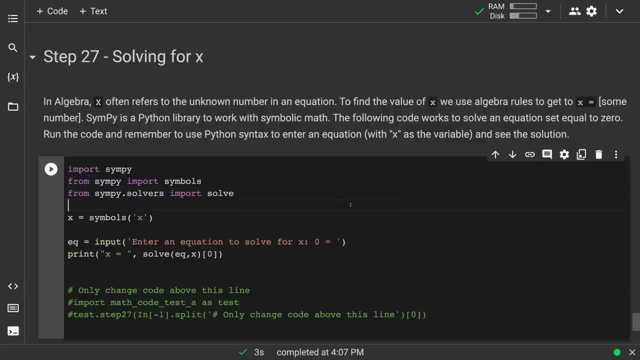 going to import solve. So all these. now I'll just define it here: x equals symbols and notice it's just x in single quotes. So that's telling us that we're gonna use x as a symbol in math. And the way that SymPy solve works is the equation has to be equal to zero. 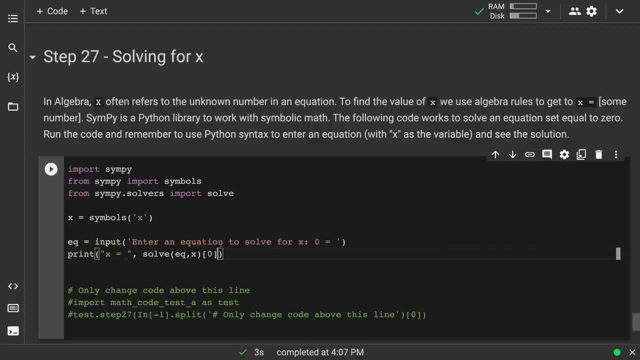 So you're going to import solve, And what I'm going to do. all right, well, see, here's the output: solve for x, and I even have this here: zero equals. and then you're going to enter it in. Now what this does. SymPy has this. 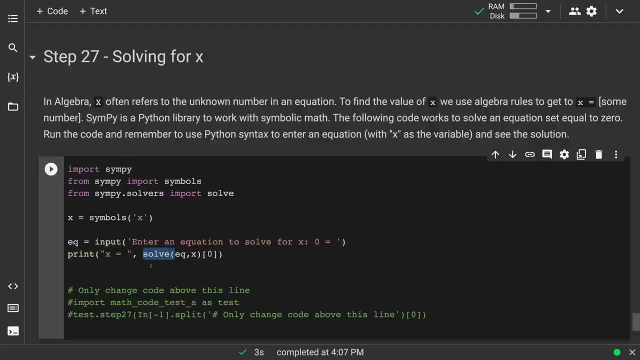 built in: solve And notice the output is going to be right here. So that solve. we know that behind the scenes it has a return value. So solve that equation using the variable x. And this is just like a subtle thing that we will talk about at another. 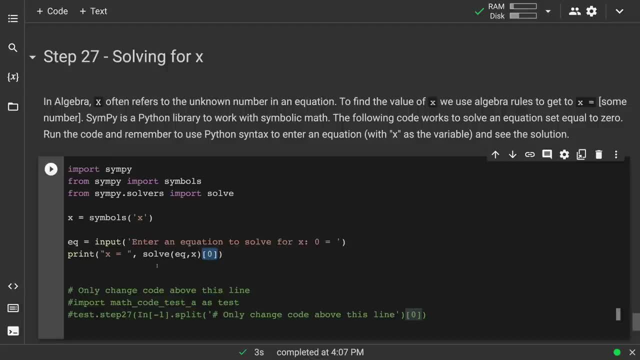 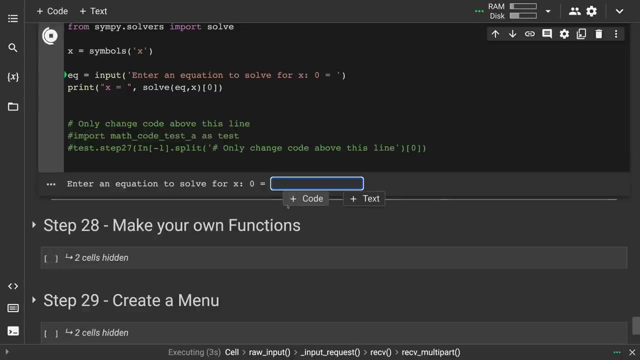 time. But this returns a finite set And for this we're going to say- this is the first answer that we want, equation zero. So enter an equation and then this is going to output the answer. Here we go. All right, And an equation, and so, if I have, let's do, like you know, two times x. 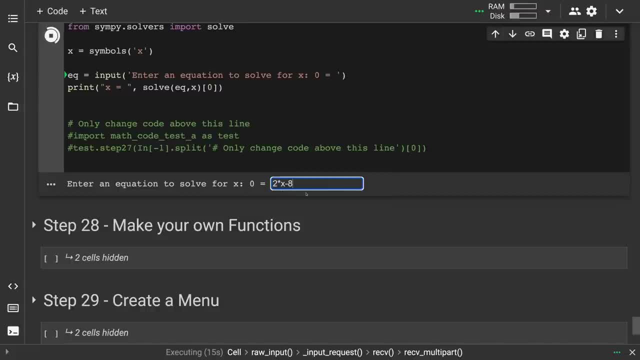 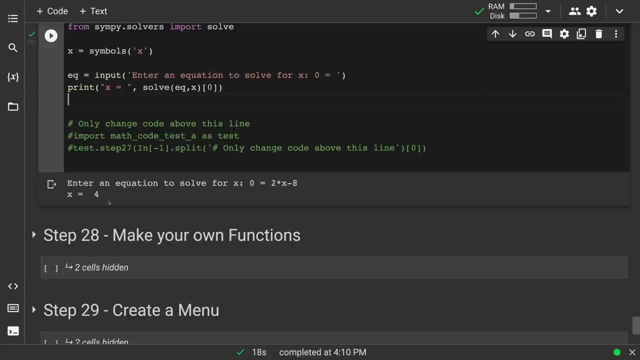 minus eight, so we can see that x must be four, And I'll put it there. Now, if I didn't have this, I'll do the exact same thing 2 times x minus 8.. Just the way it displays it, because it's a finite set. 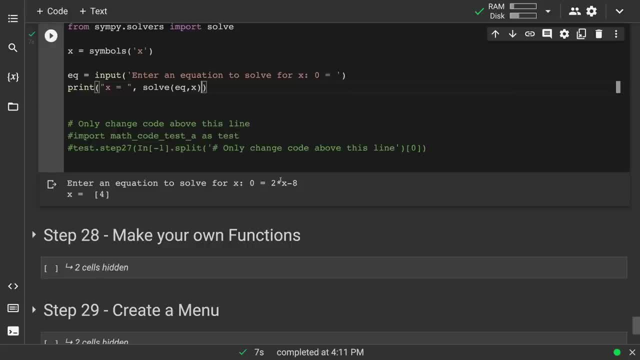 Now that also opens up the door to possibly, if I put in something that had more than one answer, I could do that, And that works too. If I have, let's see if I run it again. So supposing I have now, this will work. 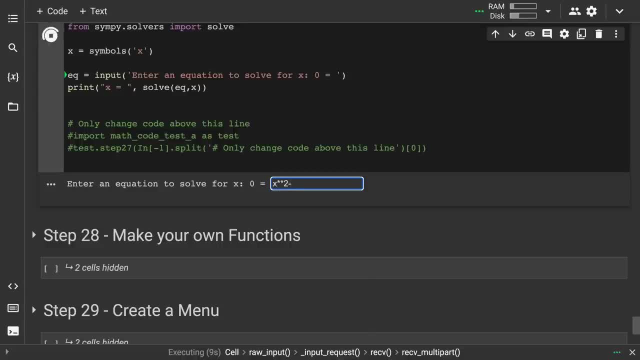 Even if it doesn't work out to a nice integer. but I'm going to make this work to a nice integer: x squared minus 9.. You see negative 3 and 3.. It does have two answers and it will output both of those. 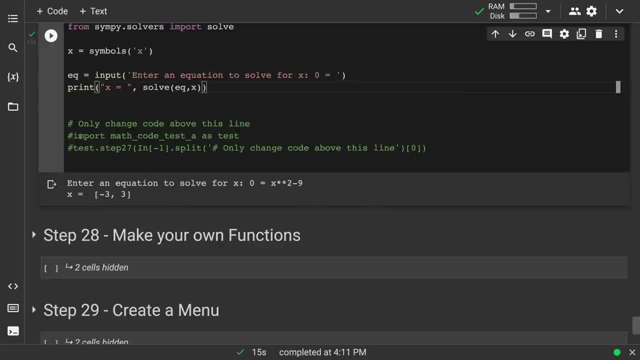 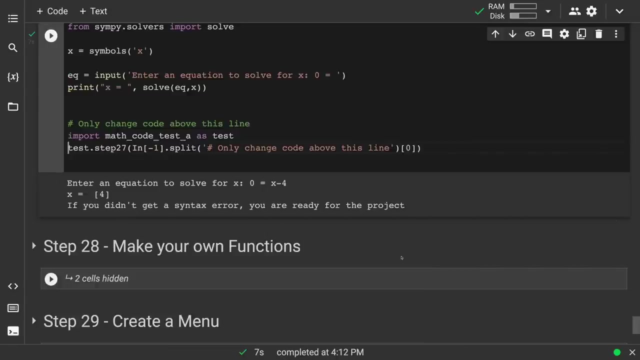 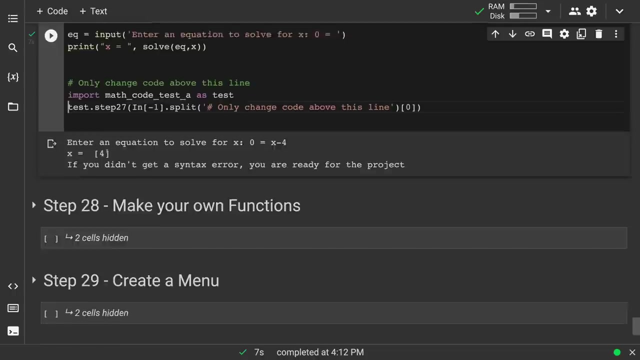 So this one: Go And Enter an equation: x minus 4.. So there we go. If you didn't get a syntax error, you're ready for the project. So different things you can do. So this is where we now can make your own functions. 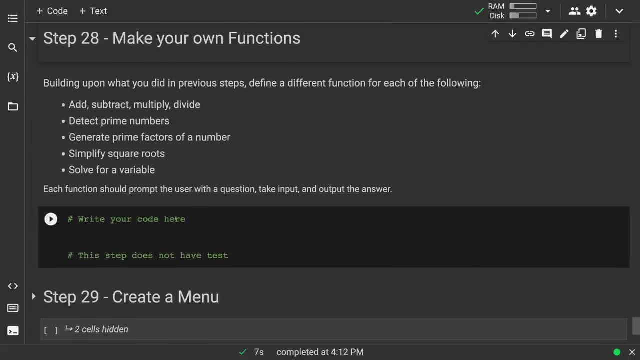 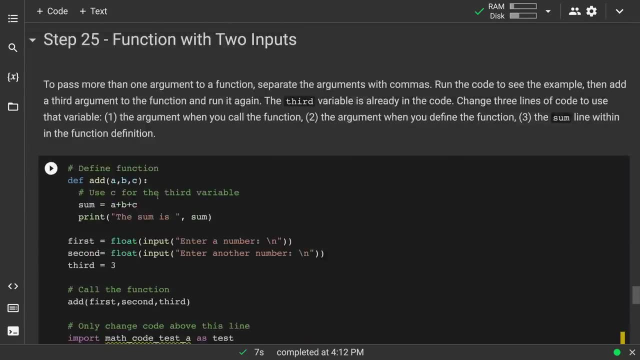 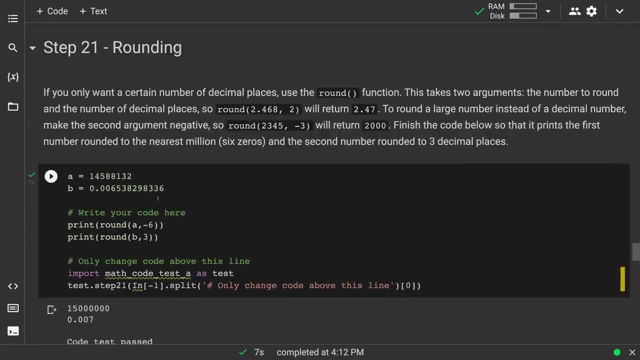 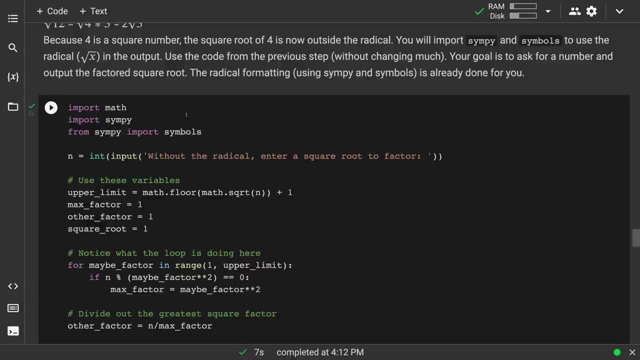 And this is where I leave it open to you How you could do this. you know, make your own functions, Like you could take one of these functions here, Like the factoring the square root. Yeah, so you could take this factoring the square root and copy all of this. 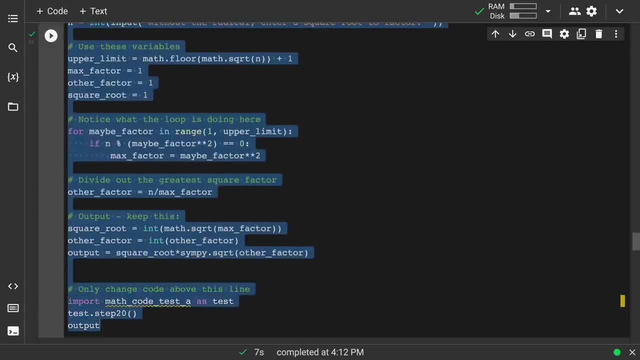 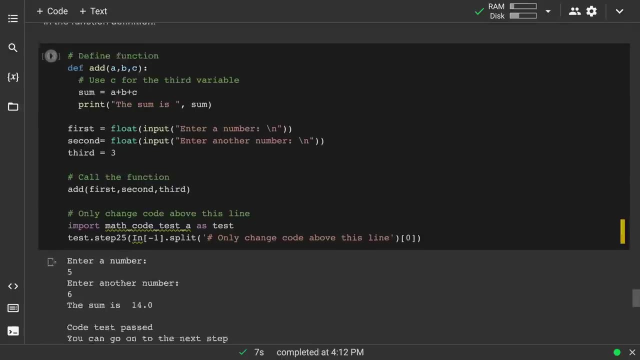 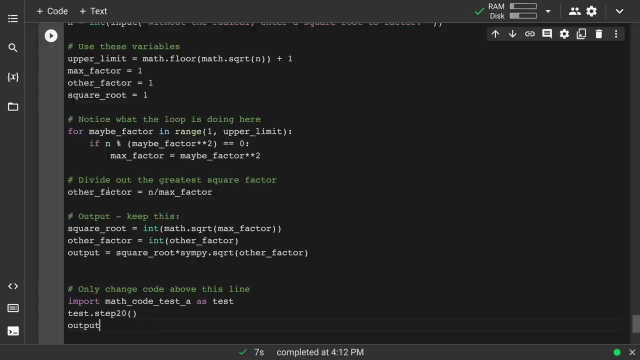 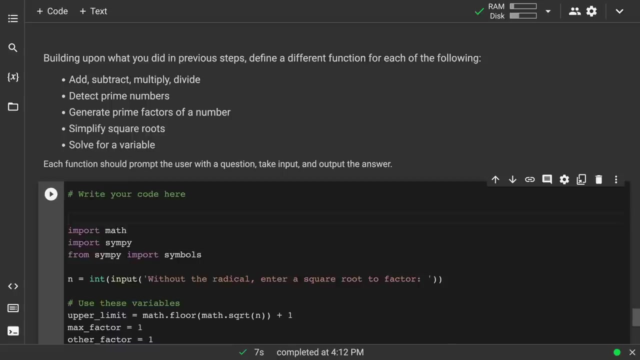 All right, So as an example of something, something you could do, and down here you could make this a function. So you could do This. now what's interesting is you as defining the function. here You could define it: Factor SQRT. 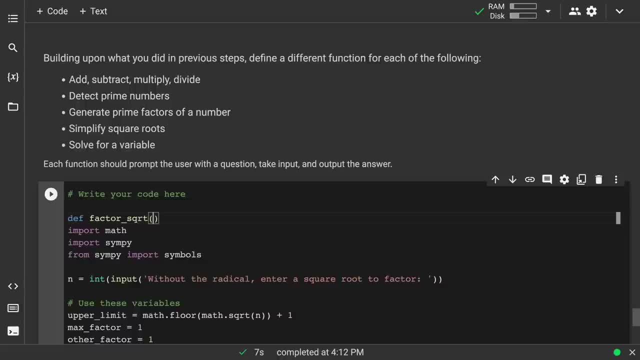 And we definitely want input And I'm going to make it in So We could do this, that It factors the square root and you could make each of these. Then you have to make sure You indent everything Now, since we're factoring square and we don't need that input. then we can actually delete that. 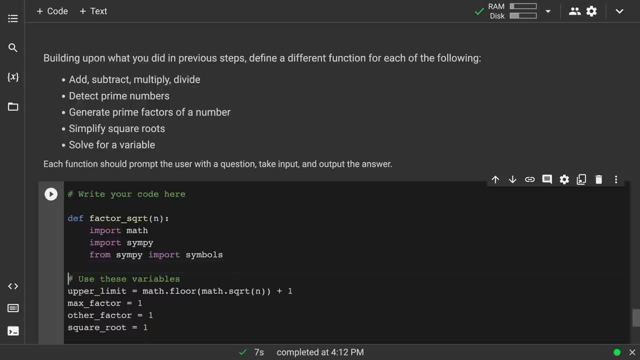 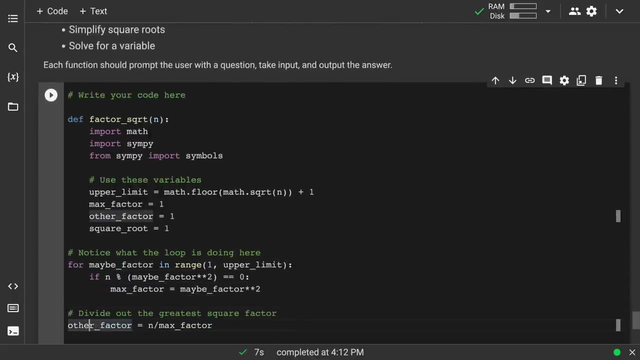 And here we go: Use. you know we can keep all these, And this is the thing with a function Is you do want everything To And you can take out things like notice what it's doing in the loop. There we go. 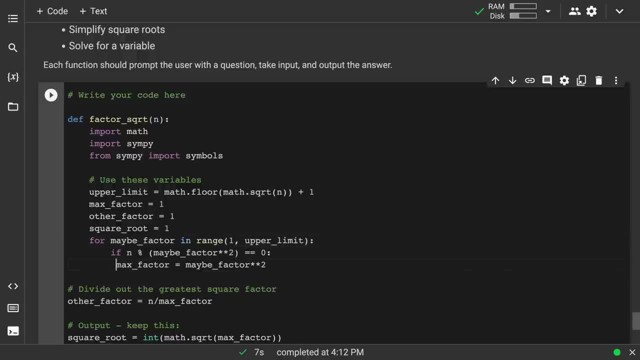 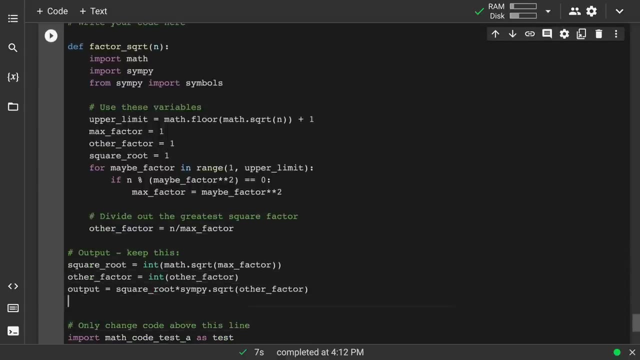 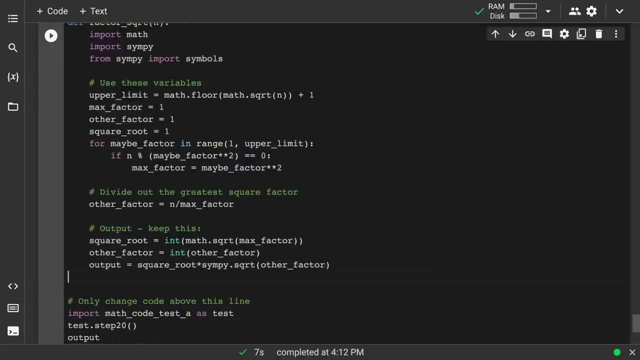 Then this has to be intended. There we go And all of these divide up. We can even keep these, And we see that we have output. Okay, All right, And this part we don't need. Um, Yeah, Oh. 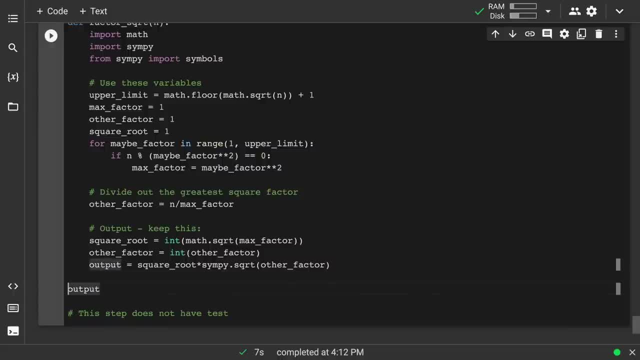 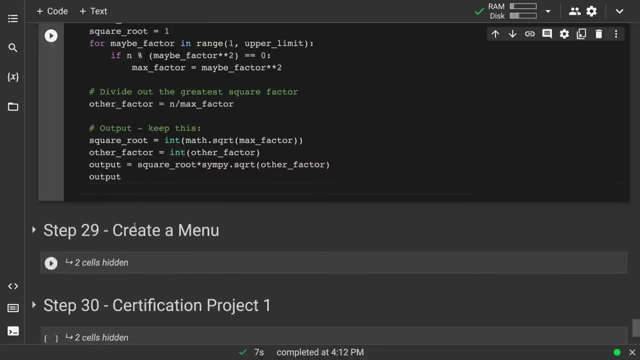 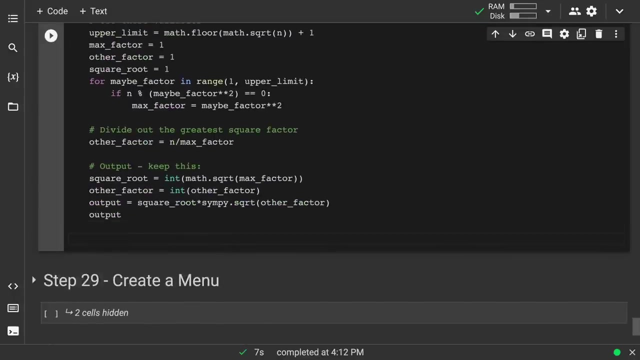 And And what do we want to do? We want to. We can backspace that, Okay. Yes, the step does not have a test, because this is so. what you have is you can define that factor square root and then down here later. 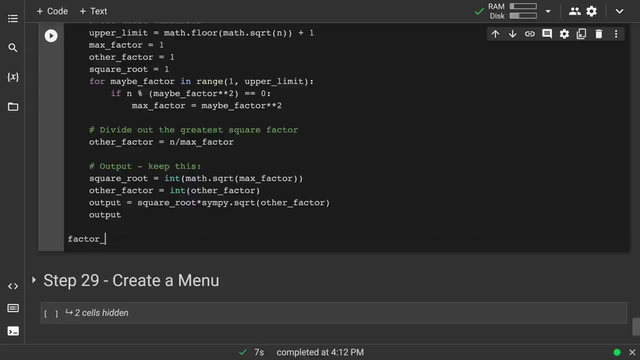 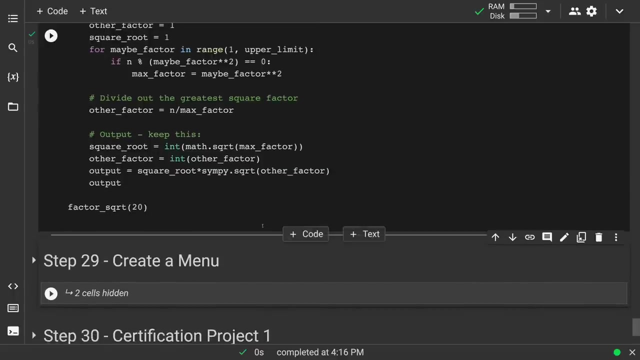 We could try to call it Factor, Factor, square root, and you know, uh, let's see um 20.. Yeah And Oh, maybe I have to return the output. It's actually kind of funny That just popped up. but there we go. 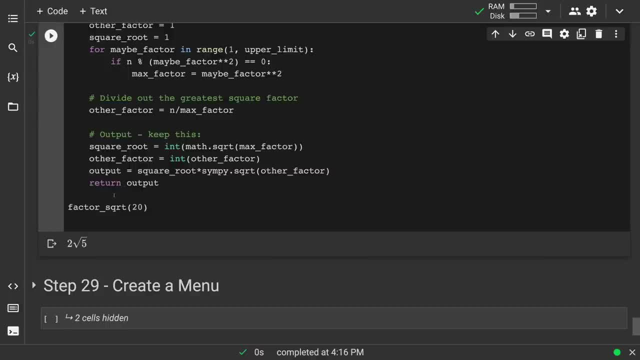 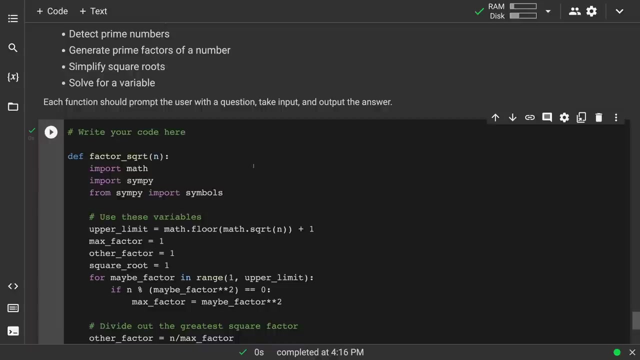 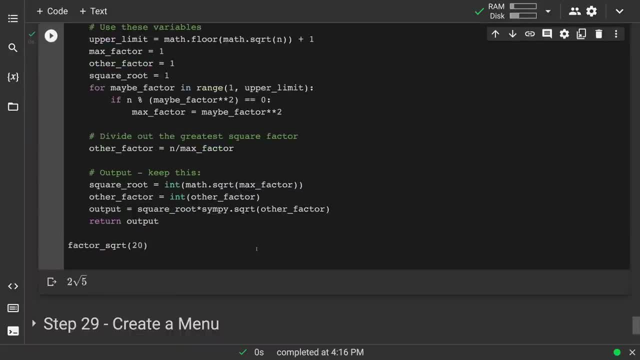 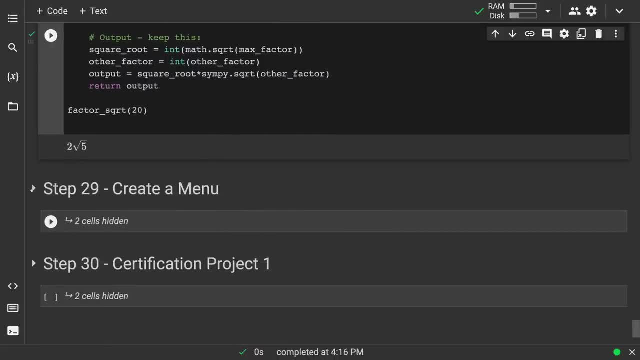 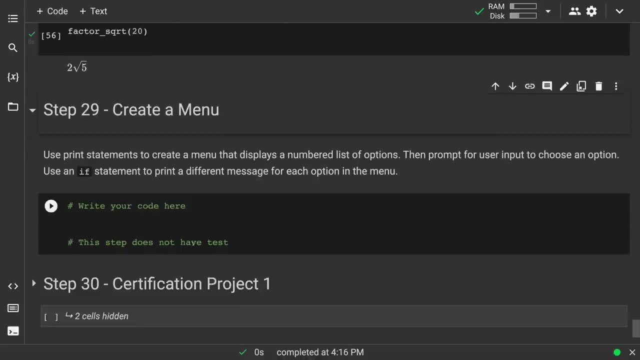 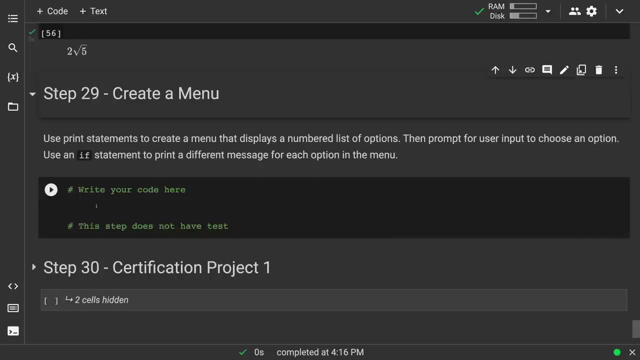 You could make them all functions, Um, but that's the idea. And then you could create a menu, if you wanted to, where you just have um, which one. you know what function should you run. You could do a table of contents there too. 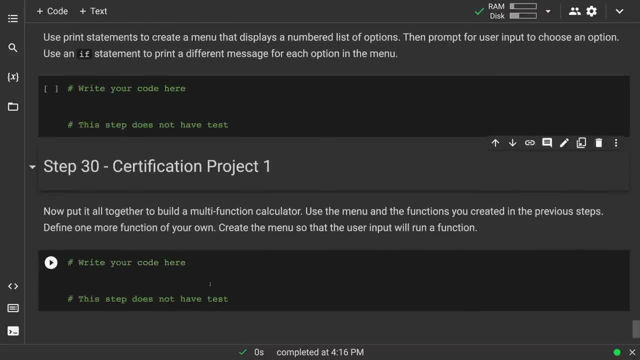 and then that's the, that's the project. you're building this multi-function calculator. you're putting all these things together into a colab notebook that you're going to be able to use, and it's going to be your multi-function calculator. and then, as of making this video, i can't tell you exactly where to upload that, that code, but hold on to it. 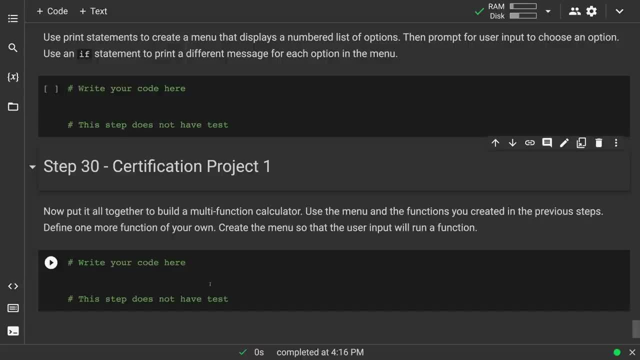 and then you'll see where to put it together, for you know, officially, uh, getting the credit for passing this part of the certification and then maybe on to the next part. all right, so hopefully this was useful. um, you know how to work through this and how to um put all this together into. 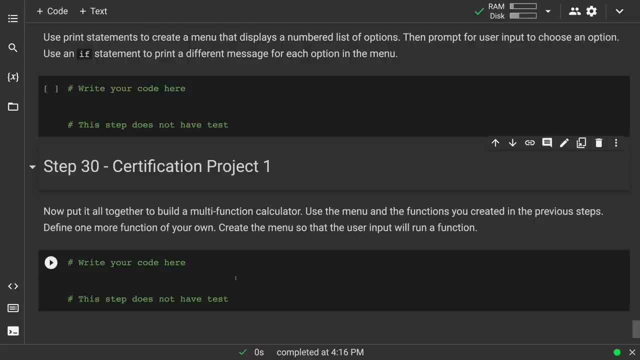 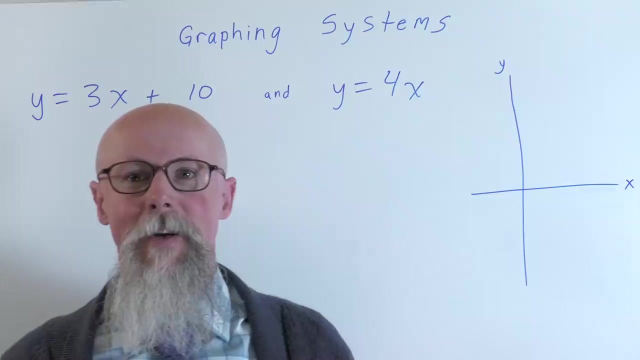 this certification project, and you know we want it to be. you know that there's more than one way to do all this, so find, find a way that works for you. you know making your own calculator, all right, and we'll go on to the next project. so with graphing a system of equations, we're looking at really just graphing two equations. 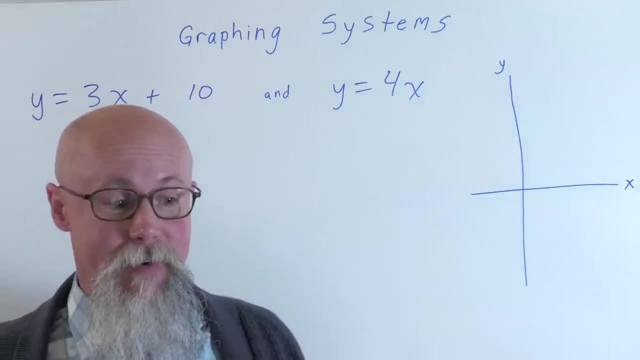 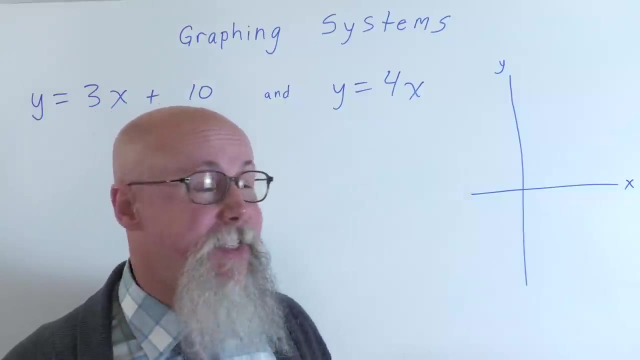 on on the same x- y axis and we want to see where do these two lines cross. that's going to be the solution to our system of equations. so, as an example, here we have two equations, and this one's y equals 3x plus 10. 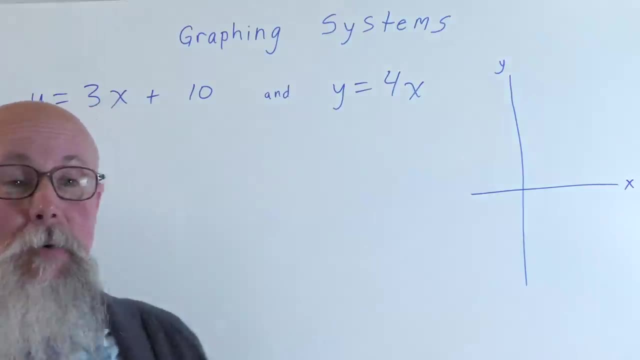 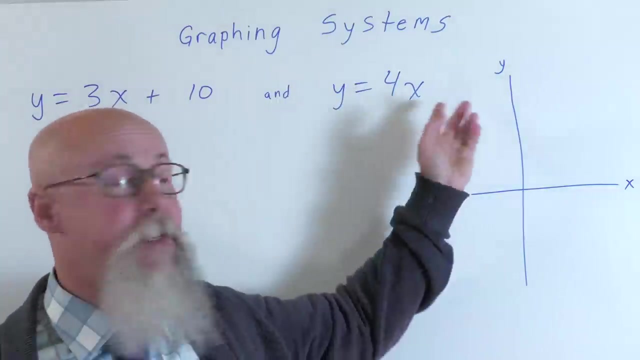 and this other one's, y equals 4x. so let's say: i don't know, it's um place you like to go. let's say costs: you know four dollars admission, so four dollars times x, which is every time you go, then y would be the total cost and then they have a deal. oh, 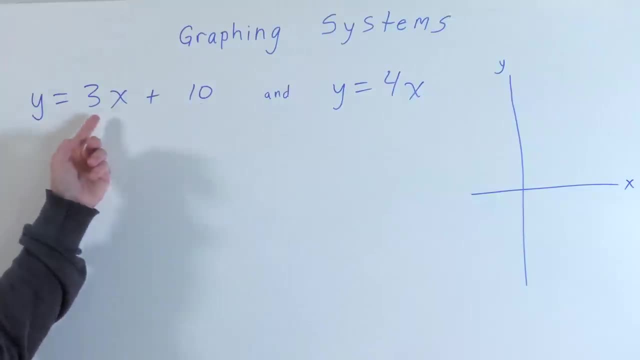 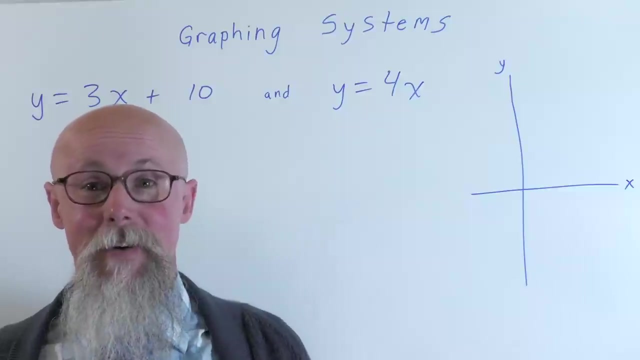 well, if you pay ten dollar membership fee, then your admission's three dollars. so there you have the, the decision like: okay, well, with this membership fee, my admission's lower. but when would these be the same price? you know at how many times would i have to go for these to be the same price? 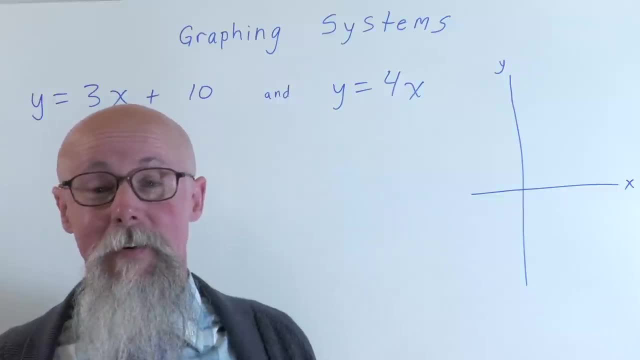 so we want- you know, that's just one example of the of you know the use of this, so i put these together and i'm gonna get into some other ways to solve this, but we're looking at just how this graph plays out here. so if i graph that, y equals 3x plus 10. so without numbers here, we're just going to estimate. 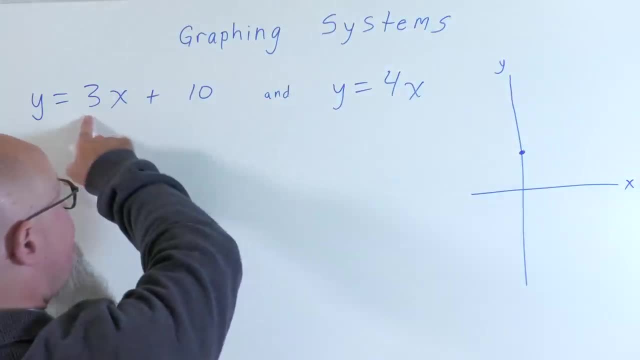 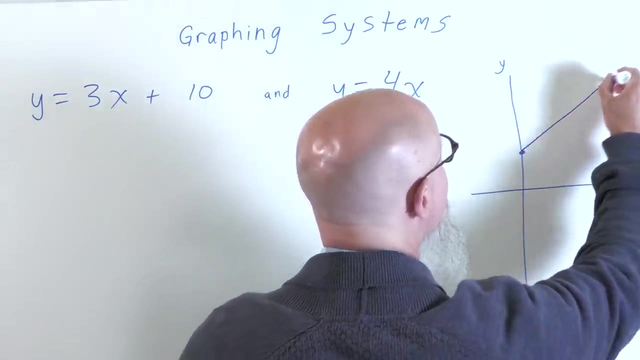 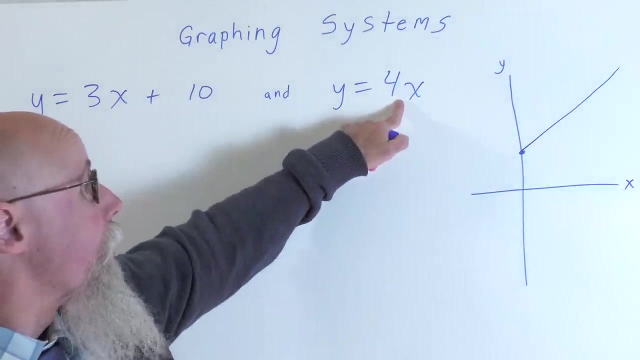 let's say 10 is here, and you know that's how we plot: begin at 10 and then up three over over one. and let's just say: you know it's something like this, and let's just say that's the line, and then we have y equals 4x. so 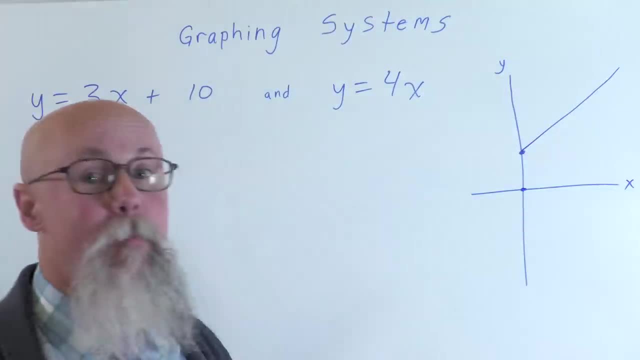 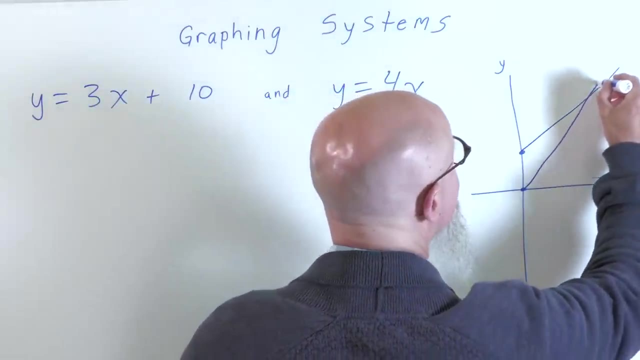 So there's no beginning, it begins at zero, but it's a steeper slope, you know, be it zero, steeper slope. And then let's just say, you know, it looks something like this, And then they cross somewhere. 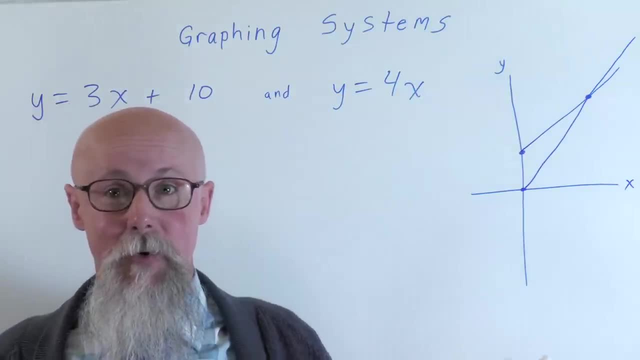 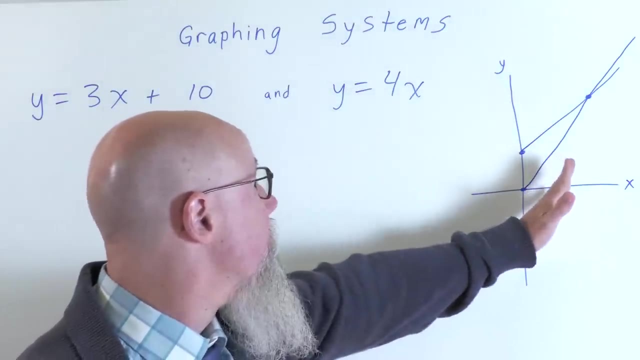 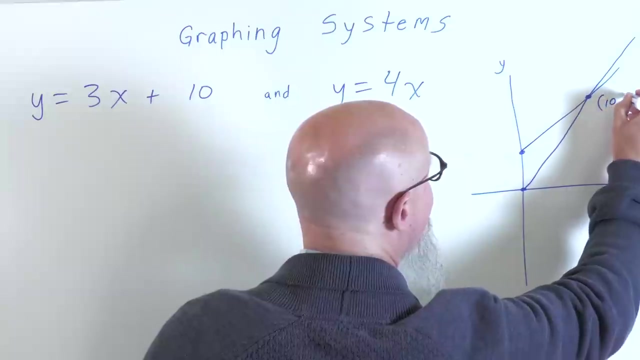 Where do these lines intersect? That's going to be the solution to our system of equations, And let's just imagine that there are numbers here, and it was, you know, somewhere around 10.. And so you know, let's just say that that would be like 10,, you know, 40,, something. 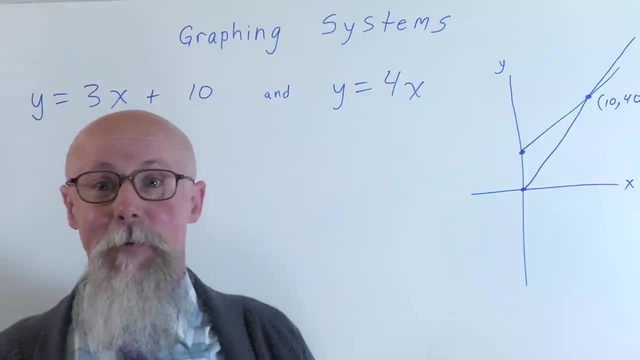 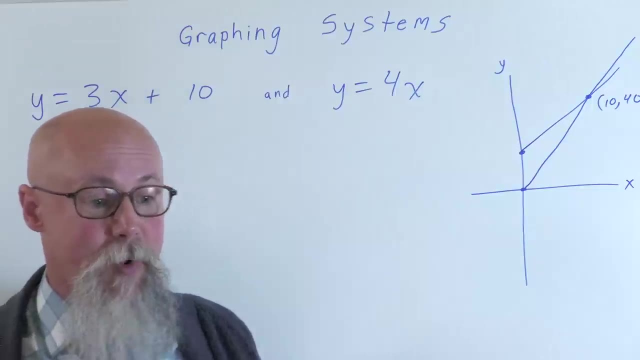 like that. You know, I see the invisible numbers on there, So you see where these cross and depending on what you're using to graph, you know it might be clearer to see, might be harder to see, but we can then always test it. 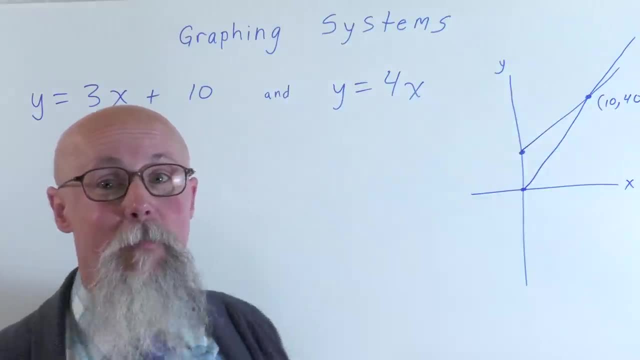 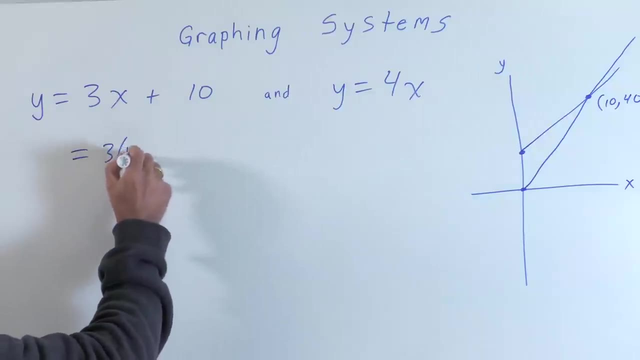 Oh, if I see it looks like that's where these lines intersect, we can plug that in. Does that work for each one? So if X is 10,, so it would be 3 times 10 plus 10, and then Y would be 40.. 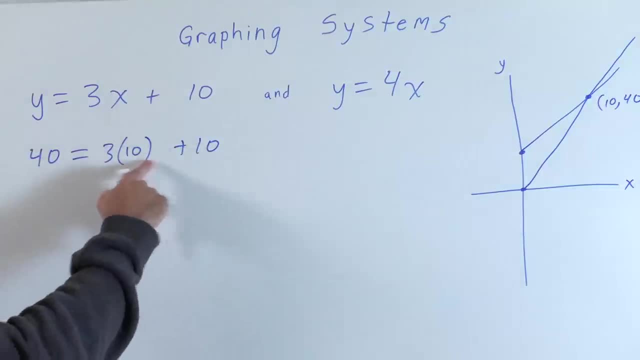 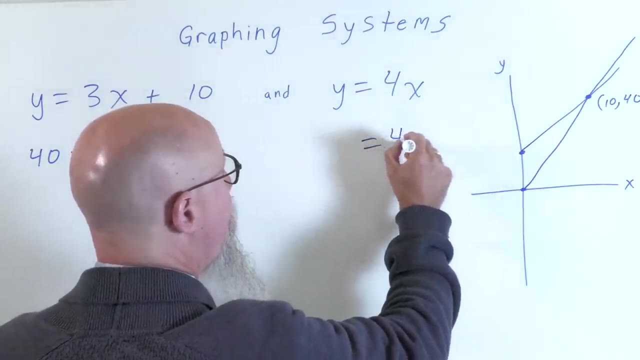 So our question is: does that work? 3 times 10 is 30 plus 10 is 40.. Yes, that does work. And then it would be the same thing. you know, 4 times 10 and Y is 40.. 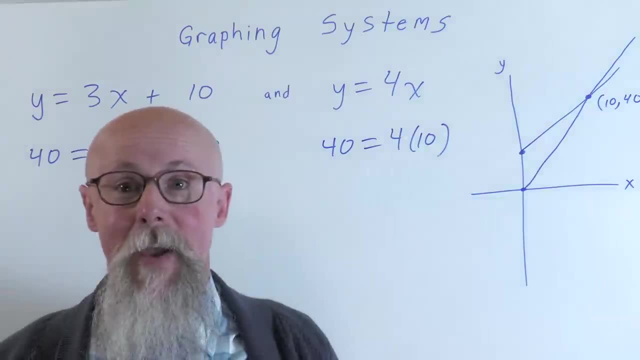 And then that works. So that's how we would confirm it. And if we were doing this, you know old school, plot A bunch of points. I could always put you know my X, Y table and plot a bunch of points. 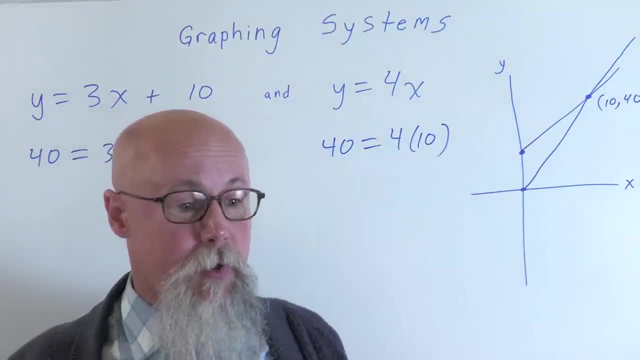 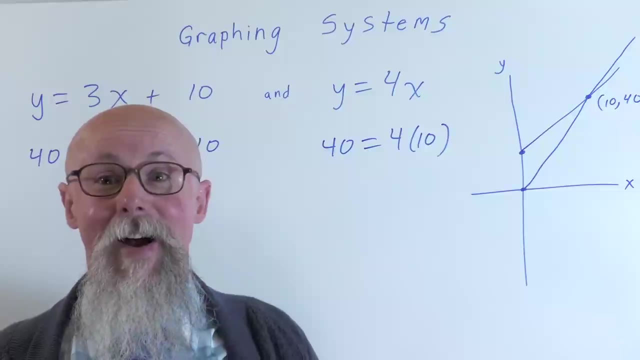 If I was using graph paper, and what we're going to do, though, and the reason why I didn't worry about getting this, you know these exact details. this is not drawn to scale- is because I want to, just you want you to see. you know the the way that this 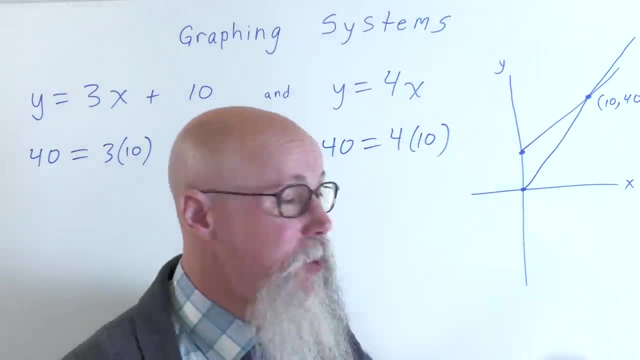 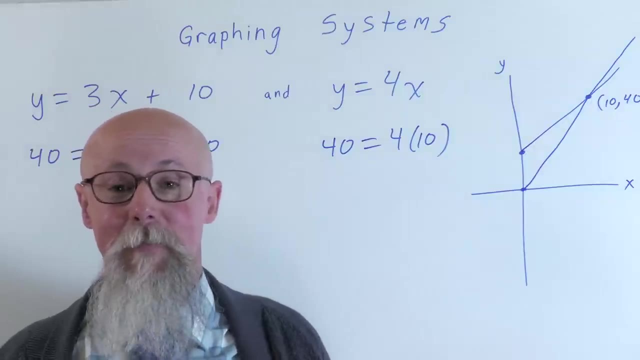 comes together to lines on the same graph. My question is: where do these lines intersect? And then next we're going to look at the code. How can I set up a graph, How can I plot Two points on the same graph? and you know, for whatever the answer might be, 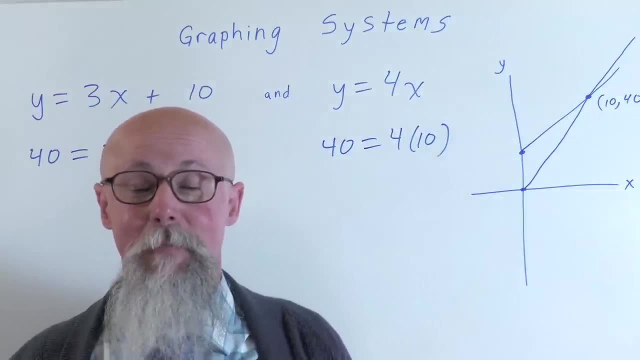 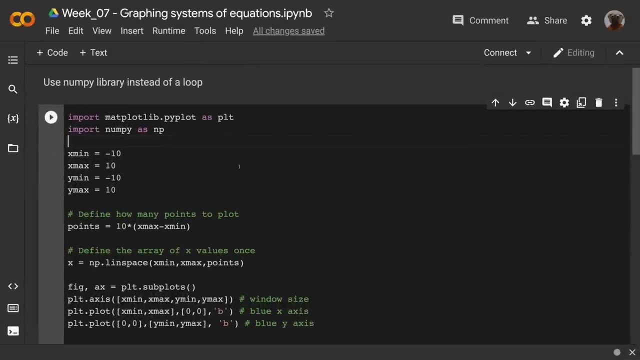 However, um, you know my new, the fraction, or decimal, might be how we can find the solution each time. So now let's take a look at the code. So if you remember graphing one equation on a on a Cartesian plane, this isn't going to be that. 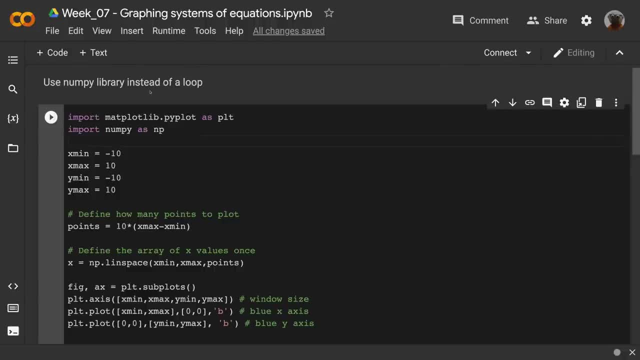 much different. Uh, one of the big things, though, is we're going to use the numpy library instead of a loop, So we'll talk about that more in a second, But the first thing we need to do is import it here: import numpy. 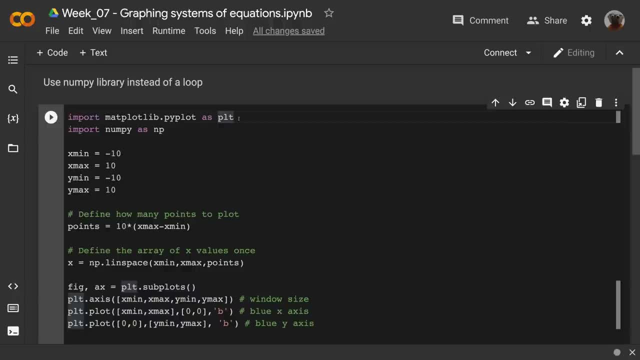 Now, you know this PLT. that makes it a lot shorter. instead of writing matplotlibpyplot, numpy, we shorten it. You know, it's just a little bit shorter, but NP seems to be the you know the common abbreviation. 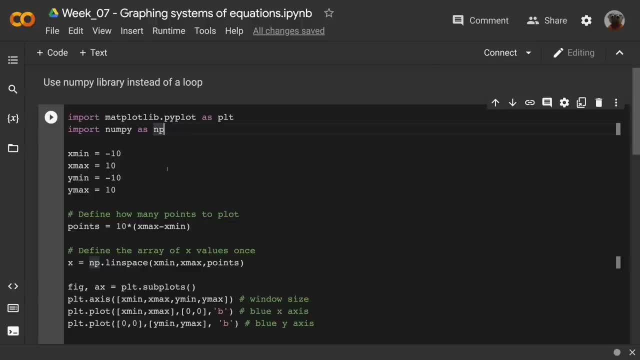 So we're going to do that and you'll see NP, dot this and dot that, um, throughout, throughout this code. So, Like before, we are going to define our range: X min, X max, Y min, Y max. There we go, And one of the things with the numpy array is, instead of creating a loop like we were doing before, what this does is this: 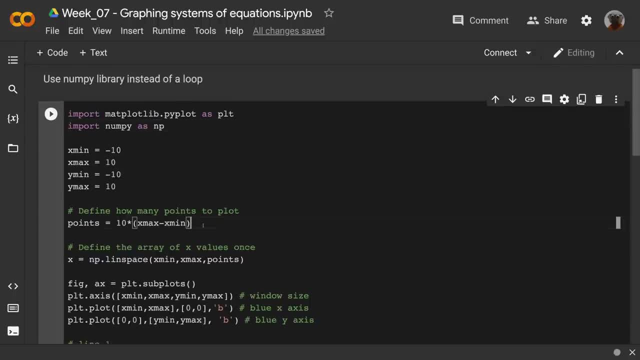 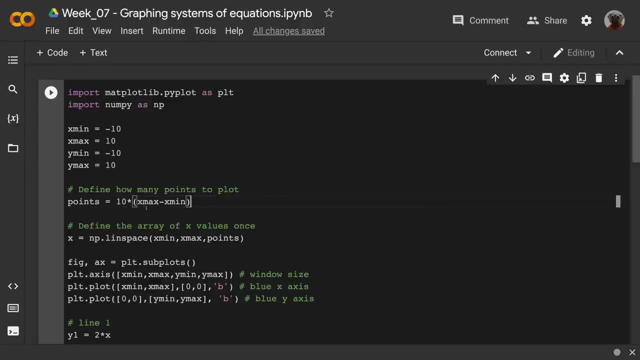 defines an array of X values, And the first thing we need to do then is define how many points I want to plot. So I'll take these X values, you know, notice X max minus X min, So how many Values I have there, and that should give me an integer number, but I'm going to say 10, you know, 10 times this number. 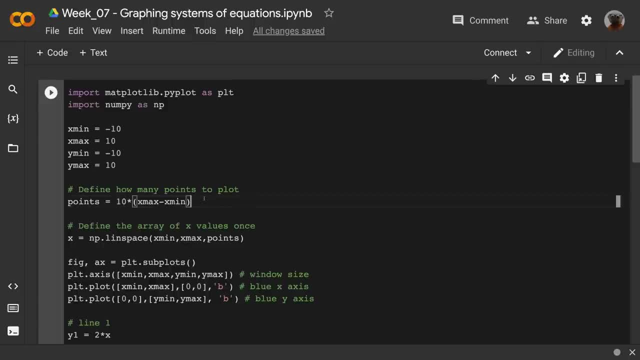 That's how many points I want. That's actually going to be for linear equations. You really don't need that many. They it displays very nicely. for anything with a little bit of a curve on it, That's probably plenty, And for some more complicated graphs you might do more than 10.. 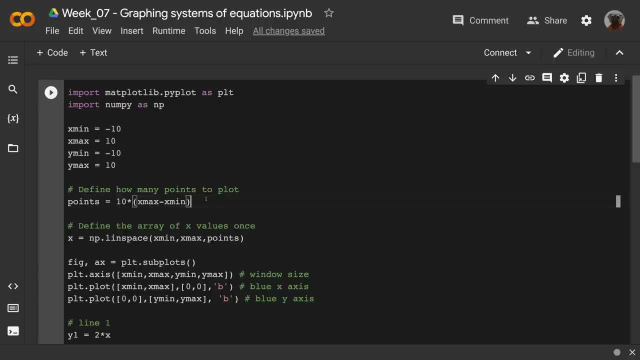 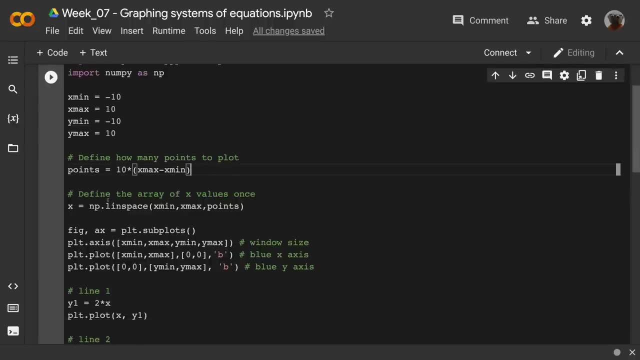 So that gives me the number of points I have, And just again based on these, So if I change the window, then this updates automatically. And then here's where I'm going to define the array of X values once. So, using that library, NP, dot, Lin, space, and it gives, it takes the arguments X min, X max, and then how many points. 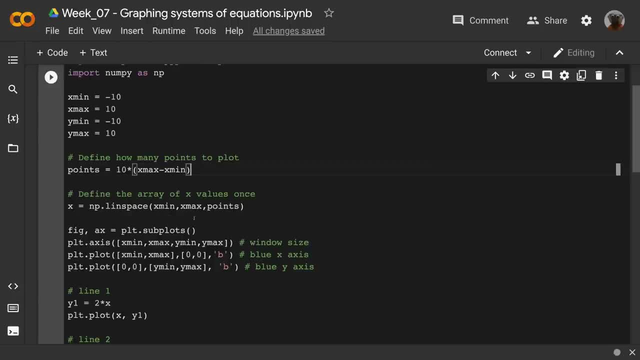 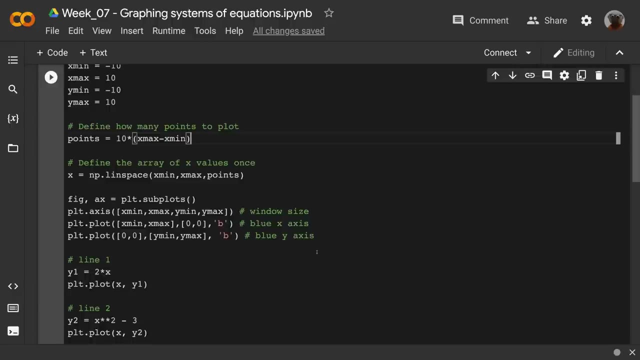 So there we go. It's just going through these: Where am I going to start and and how many points in between? and I'm just storing that as X because I'm going to use that as my X values. Hopefully this is looking familiar. setting up, you know the window size, the axis for X and Y, and here's where we're going to plot line one. 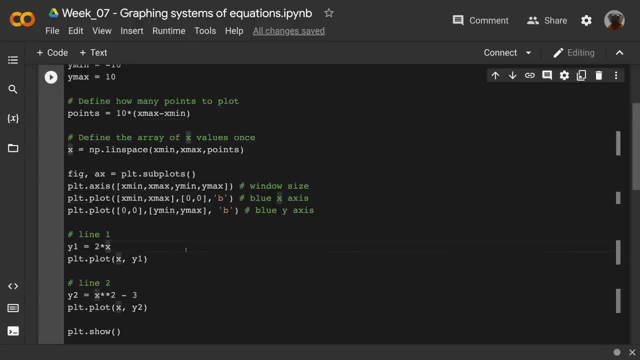 So in this case, I have Y. one equals two times X. There we go, And what it does is that will take each of these X values. rather than me needing to create a loop, It'll go through each of these X values and plot them. 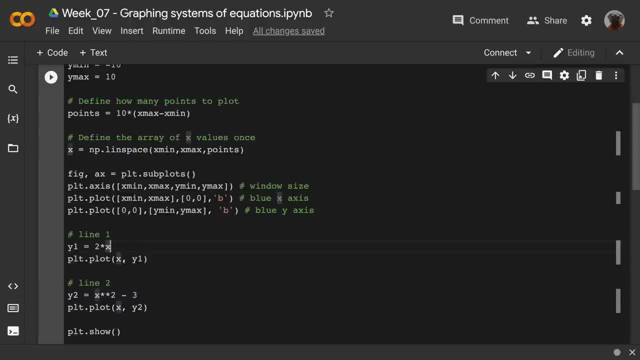 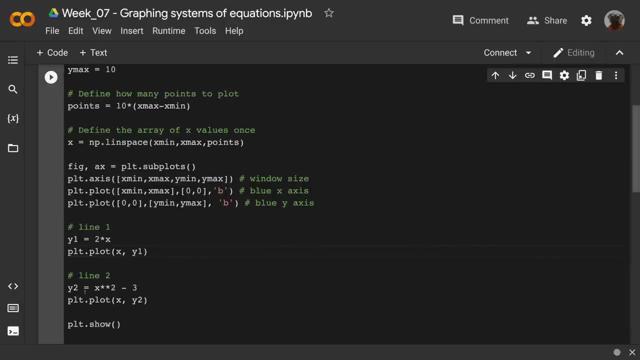 And then I have PLT, dot, plot X, and then Y one. So Here we go, I have this and the second line. I'm going to do the same thing. Y two equals and this one I took it beyond linear. 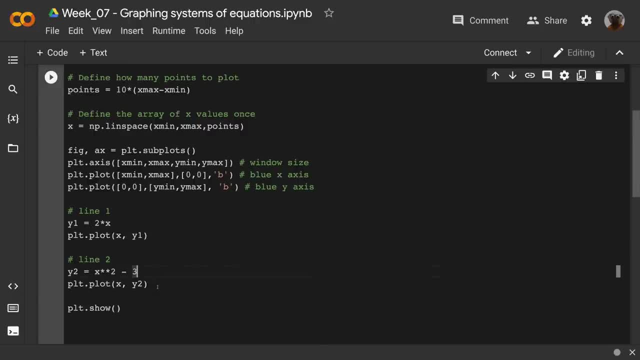 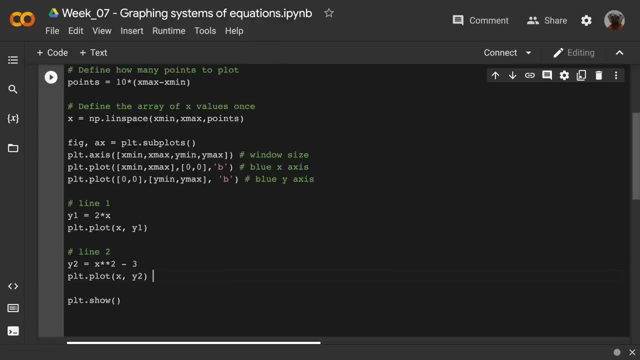 I just made it X squared minus three, just to change it up a little bit. And so there we go. That's my second Y value, And here we go. What do I want to plot here? X, the X values, and then Y two. 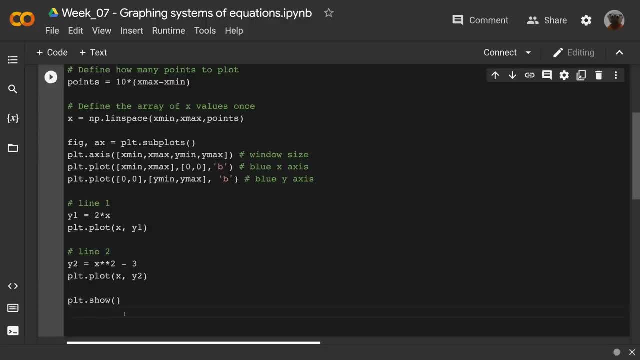 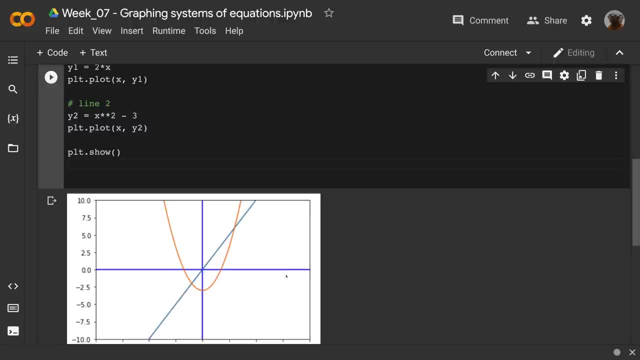 So there we go to find the X values and show the graph. So when we run this, there we have it, we have our each axis. that first, Y one, is a linear equation, light blue line, and Y two was the parabola. 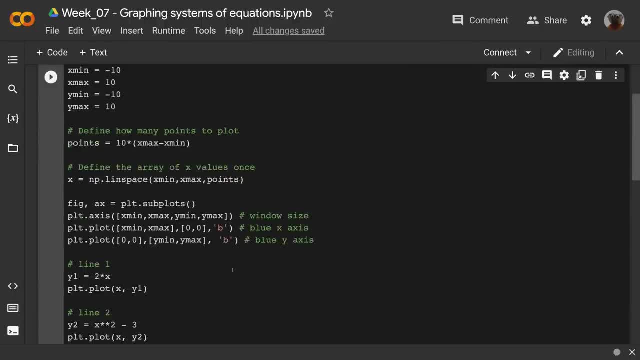 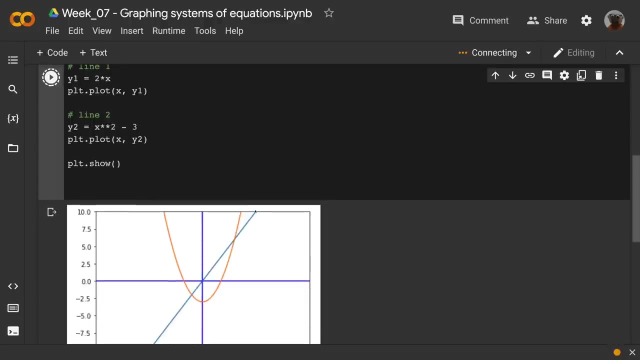 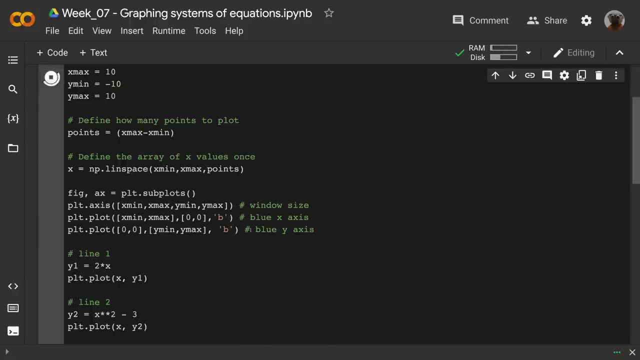 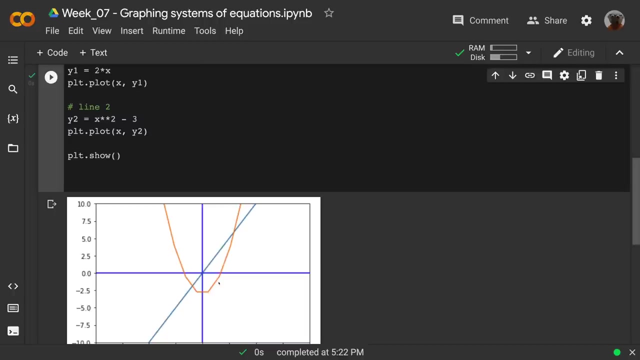 Now, that's a pretty good parabola, just to show you that if I had fewer points, let's just say even two times this, Yeah, that's probably Low enough that you're still going to see this become choppy. Yeah, it wasn't that bad. but if I really only have one times this, then it really becomes a lot choppier, because I'm only plotting every integer and there's a lot more going on here. but you see how that linear equation 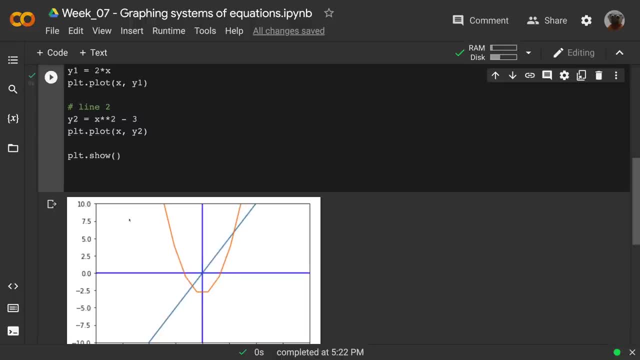 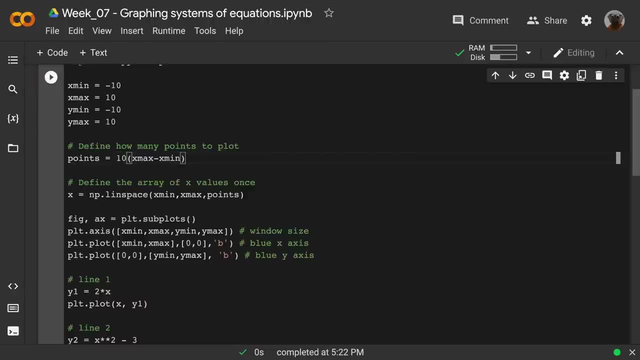 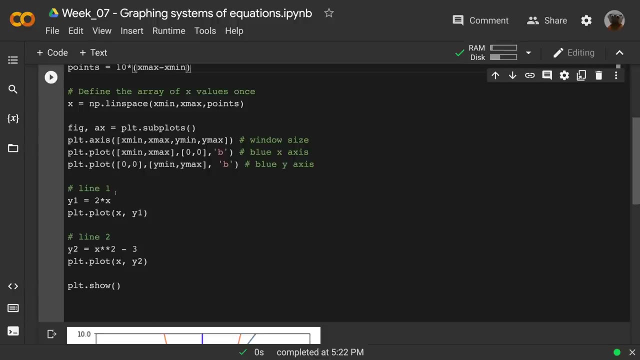 Yeah, straight line worked out just fine. but this one, yeah. so that's why, Just as a default, I'll do 10 times that, And so there we go. And then to graph anything else, all we have to do is change these Y one. 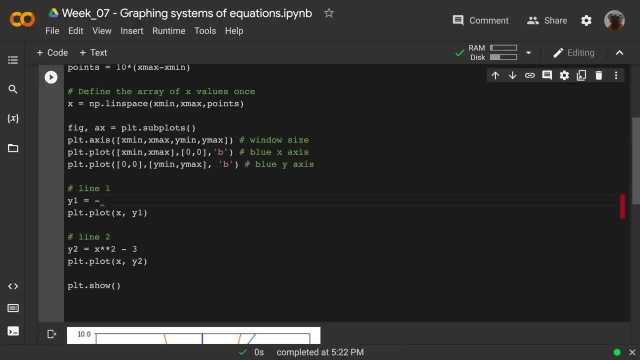 Oh, OK. well, how about if I make this like negative, Negative, three X. I'll just leave it at that. Oh, because Three times X, There we go. If you write it by hand, you know doing the math off to you know you forget the multiplying. 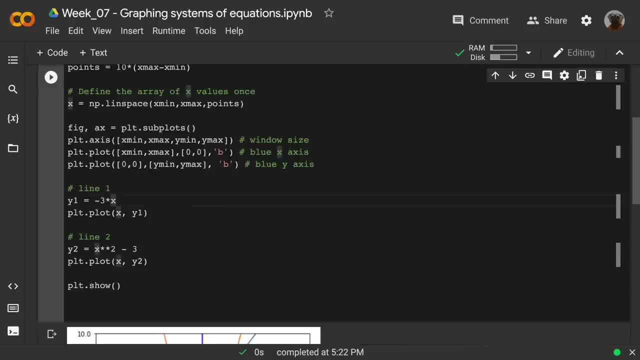 So that's the key Python syntax You have to remember. There you go. Um, and let's take a look at this and maybe we'll make this one- Um. there we go, Just to the third power. How about that? 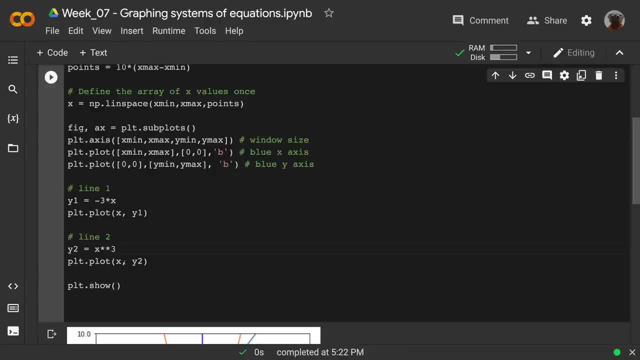 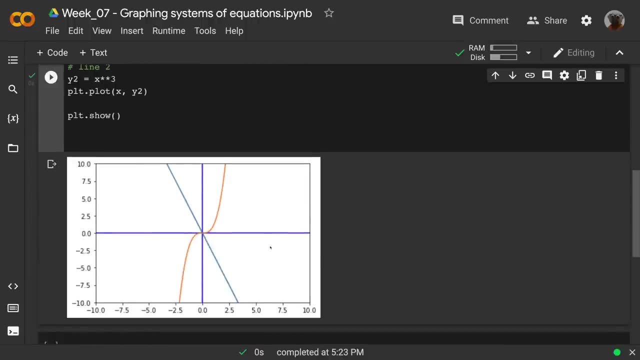 So there we go. Another linear equation, And This one here cubic, And we'll run this. There we go. And we see, You know even this, yep, the curve looks nice. So there we go, All you have to do is change. 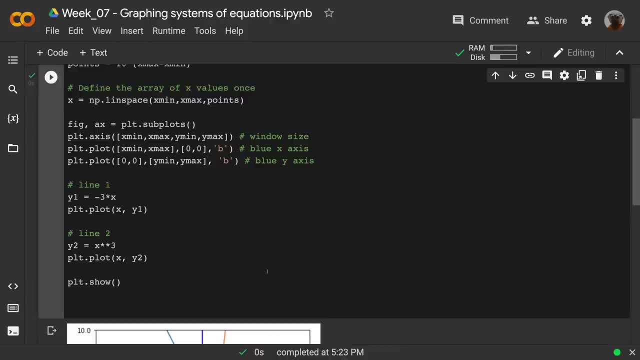 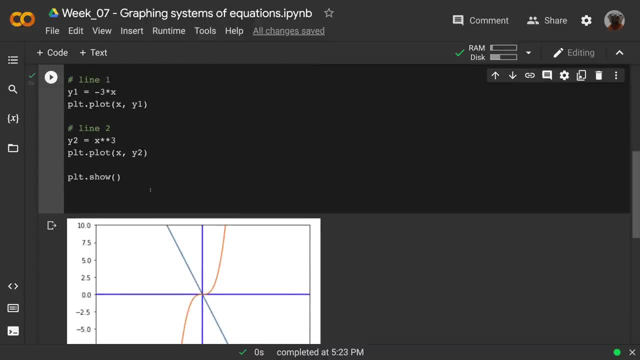 Why one and why two, and you actually can graph more than more than two. but a lot of times we're going to do linear equations and have two lines on the same And our question is: where do they intersect? So there we go. 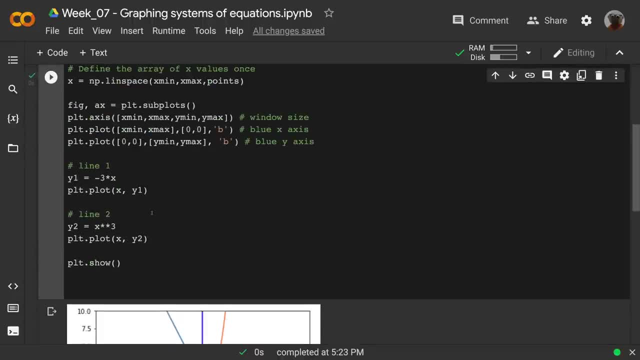 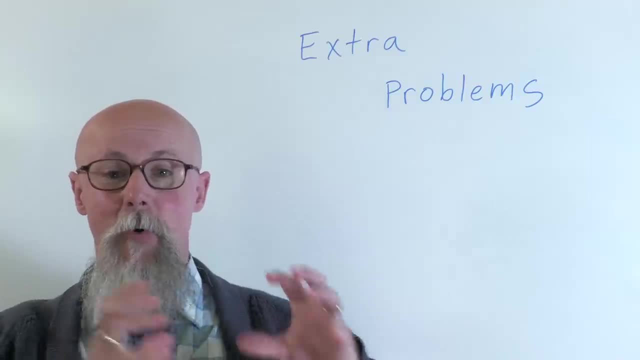 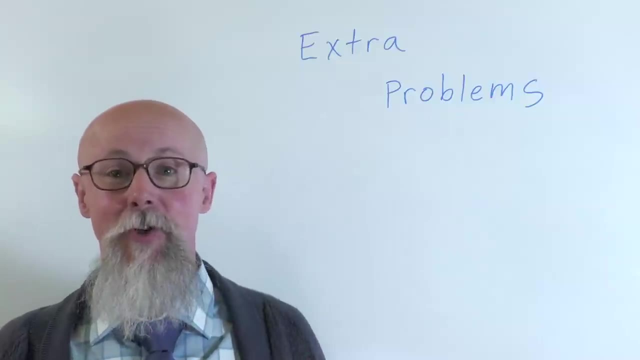 We're going to use our problem numpy and use that. Now that we've worked through the core skills in this unit, let's look through some extra problems, and I'm going to work through extra problems using the Colab notebook So you can see how you can apply these resources that you're building and use the use these to solve problems that might come up in a textbook or 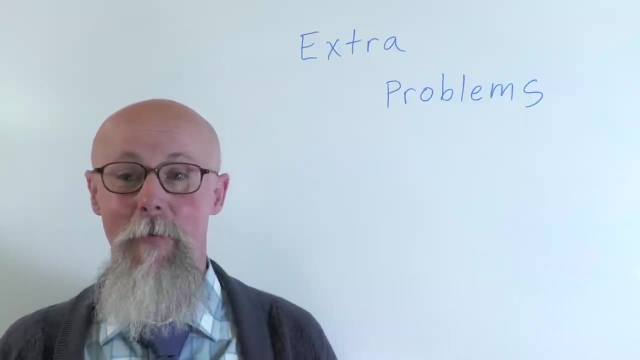 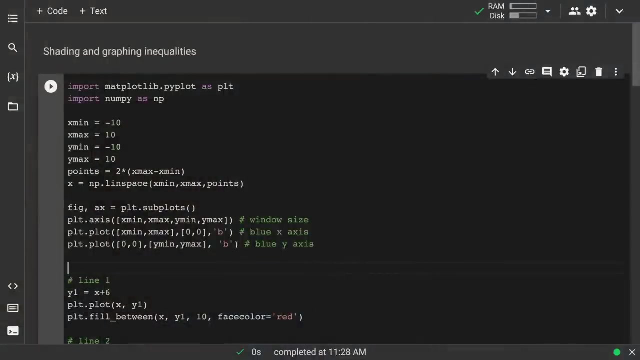 In day to day life. So So we're going to go through some more extra problems here, Okay, so I want to show you just a few other things you can do with graphing, And one of them is shading in between lines or just in general, above and below. 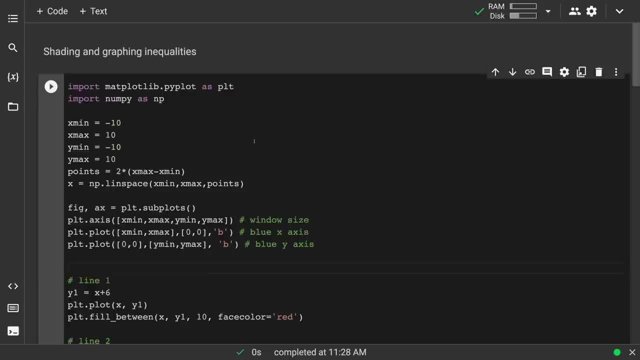 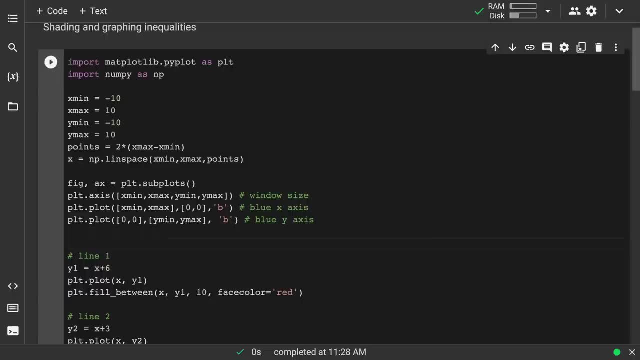 So if you have an inequality you can shade above the line or below the line. We see we don't need to import anything different. This should look familiar from the graphs you've been doing. Set up min and maximum. how many points? 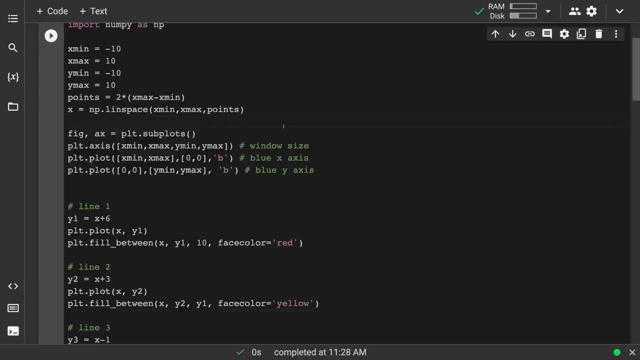 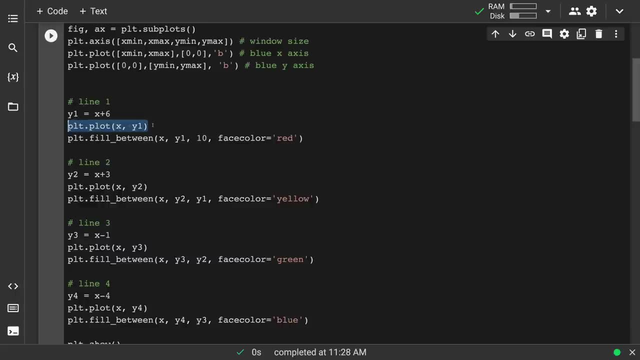 and then linspace for your array, And we've been doing this before. Here's the line, and then we're going to plot that. Now this one: if you're doing an inequality, you could also add the other argument and making it a dashed line. 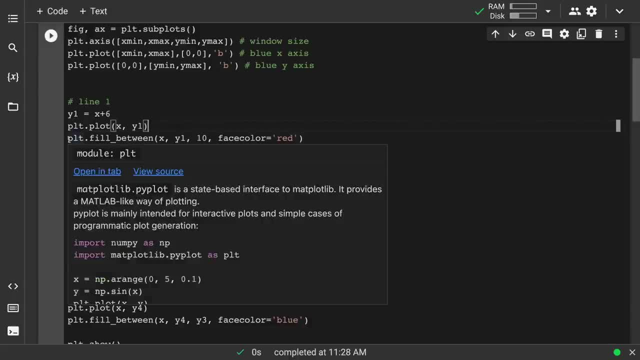 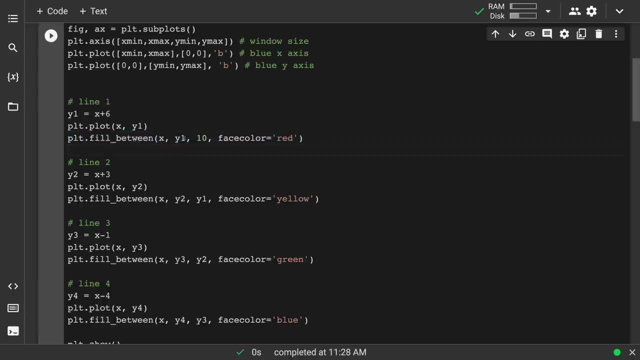 But this might be hard to see, this line, but here's the twist here: the fill between. So we're going to say from x and still the same x values, and then the fill between is between these two y values, from y1 up to 10.. 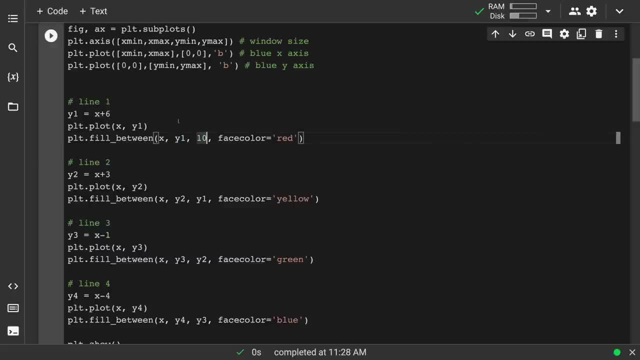 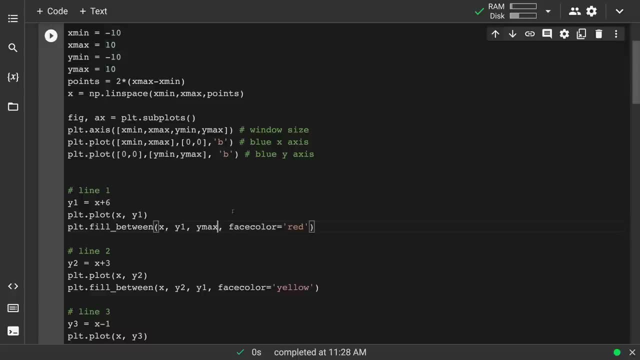 And you could define that as a definite number 10.. You know, we've already set our maximum, or you could actually say up to y max, Like that's another way to do it And this one we call it. you know, we want to make this red. 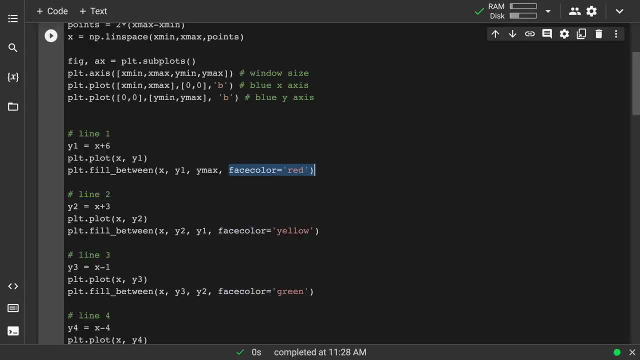 So that takes the other argument. Python will give you a default, but you know you can define these and that makes it a lot better. So there we go: The fill between same x value, and then you have the range of y values. 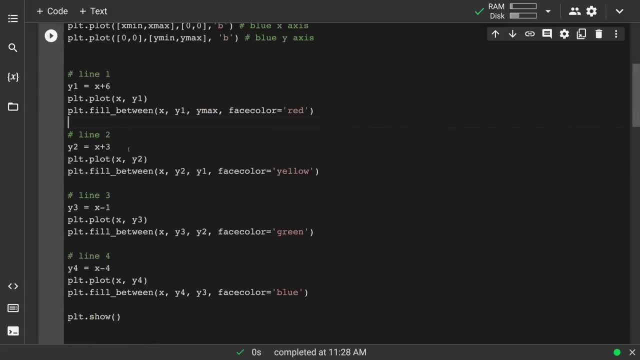 That's the way that's going to work And we'll do a few lines here. We'll make some art. So line two: you can see again the familiar, define the line and then plot. There we go, But then we're going to do the fill between. 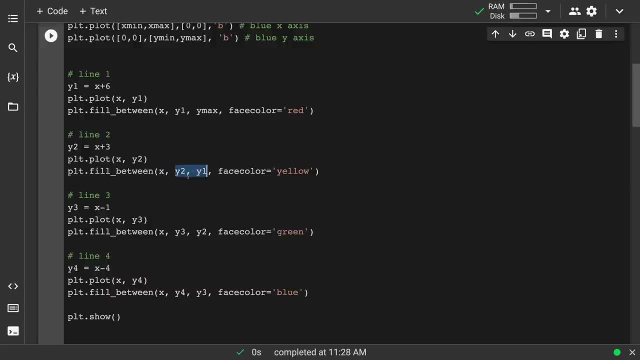 between that x and y2 and y1.. So you see, you can define it even you know. this one, I'm going to go up to the top, This one, I'm going to go up to the other line, And here we go. 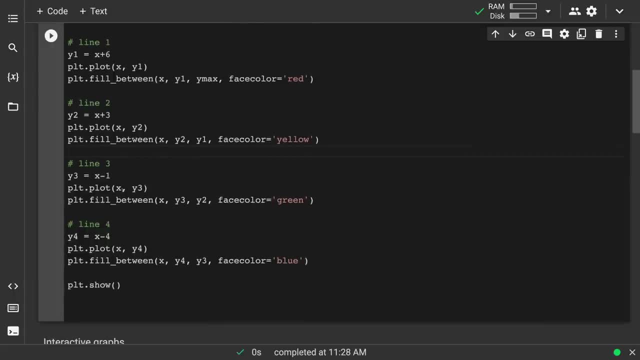 So fill line three very similar. And there we go. Each of these I'm defining a different face color, And this one's going to be green. Where am I filling between? I'm filling between this one that we've defined up here, y3 and y2.. 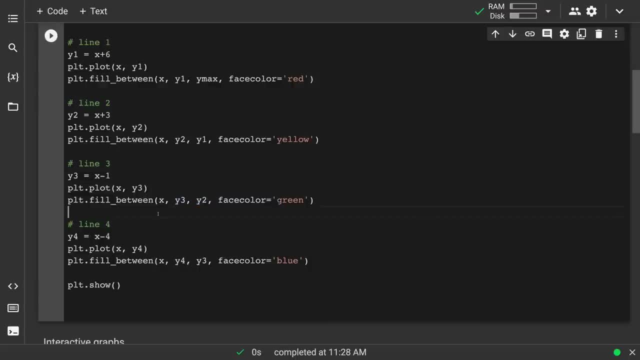 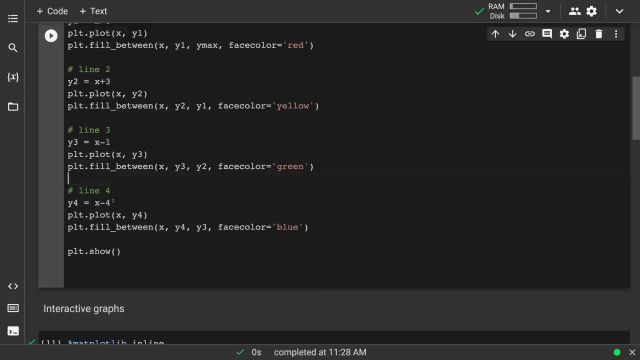 So that's so. these are just these two. line two and three are just going to be a band. and here we go. I can do this one between, uh, graphing the other one, and notice, all these are just simple linear equations to show you this, and we're graphing between these two. 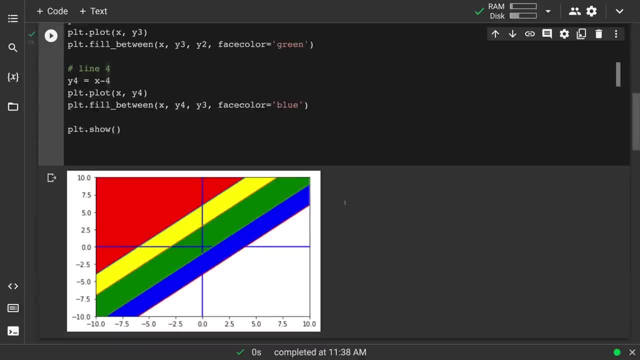 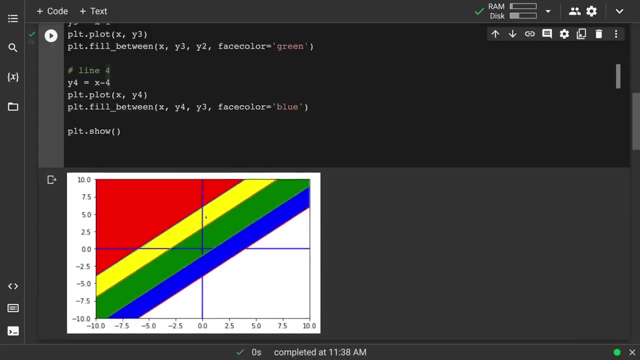 So what happens when we run this? So we see, we get the first one from that line up to the top, and then from there to there, from there to there, And there we go. So if this second one, If we had, let's say, all right, we see this red, we see this yellow. 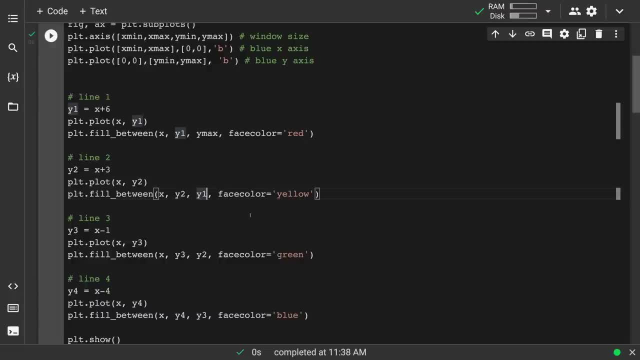 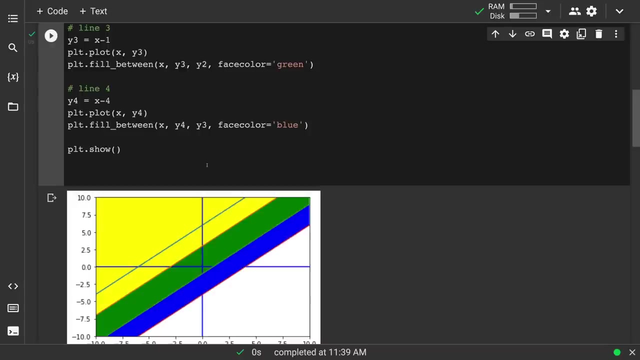 So if the yellow one, instead of ending it there, I went up to Y max, it would just overlap. And I know you might be, you might've been thinking Hey might've might turn orange. you know yellow, yellow and red, but actually it's the order of things that. 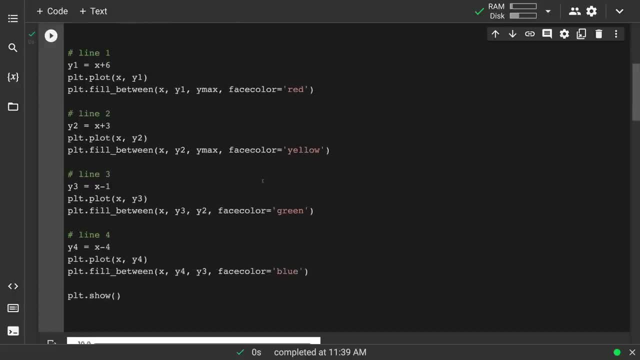 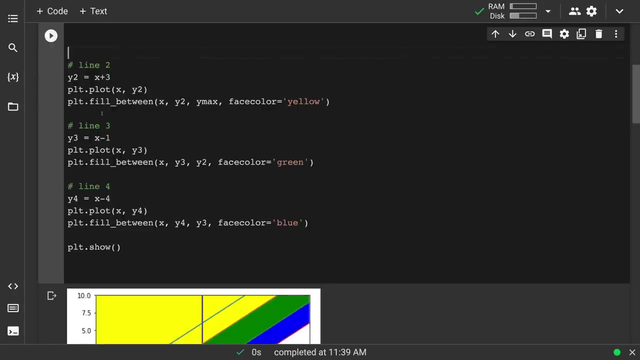 It graphs this: that was red, but then then it graphed this, and then it overwrote the red, And if I wanted to, I still caught a line one, but if I wanted to move that down here, so now this is yellow. 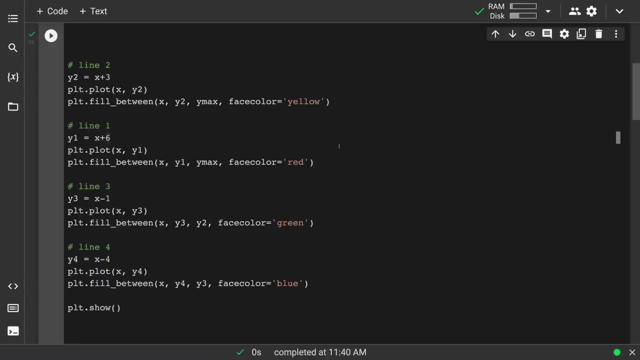 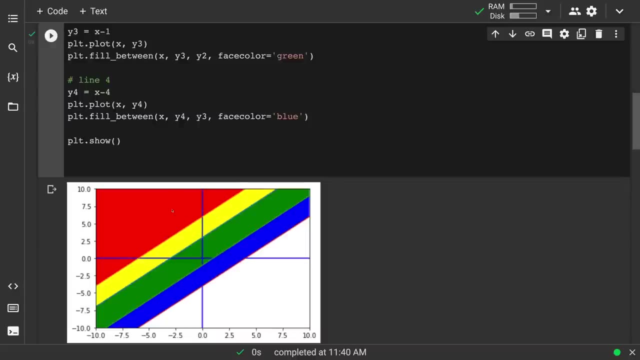 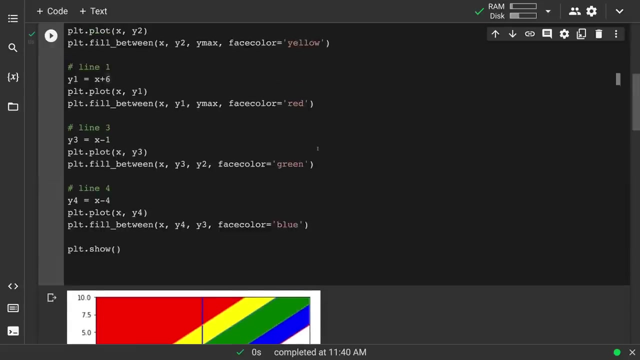 And then this whole thing would be red. And remember, Because the yellow started down lower, So the red will go on top of that, but it didn't go down this far, So the red didn't cover this. So we see, you know, that's it. 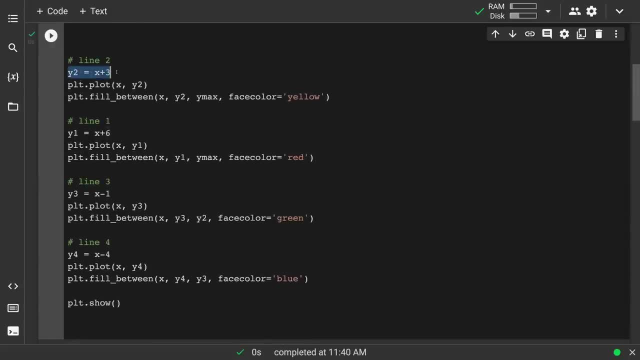 Um, you know, the yellow line was X plus three and then the red line was X plus six, So you still had that little gap that you know. when the red went on, it didn't totally cover the yellow, All right. 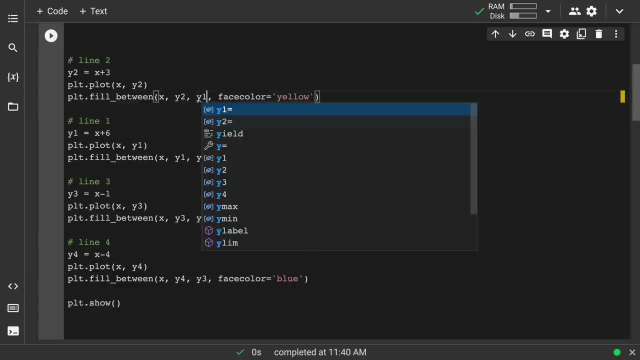 But then we can. You know why one, and now this one. I definitely need to put this one back because why one wasn't defined yet. So you see, it gave me that little error there. So just oh, I'll move it back and make this official before we go on to the next thing. 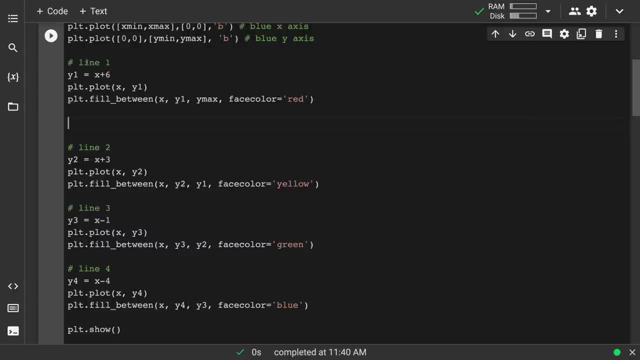 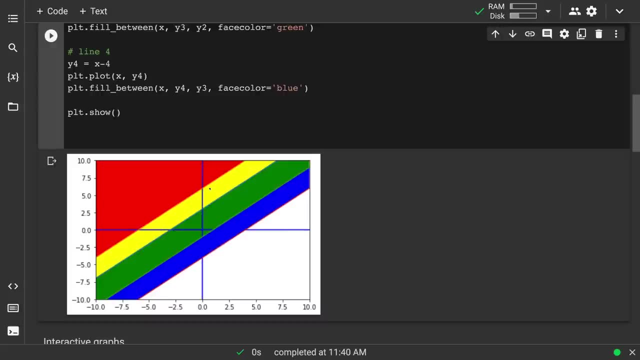 And we can see. so, since I moved a few things around before we run it, let's, let's change something else here. I was saying that we need, We could do the dashed line, So we'll make the red line and the yellow line the dash line. 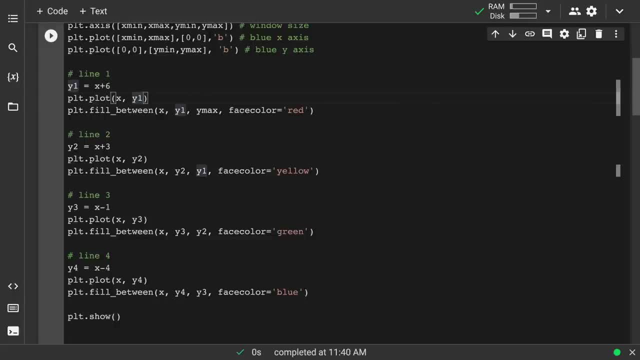 And it might be hard to see, but we will hope you can always hope here. So, single quotes, and then I'm going to make it a dash and I'll do the same thing with this one, the other argument: single quotes and I'll make it a dash so that those two would be dashed lines instead of a solid line. 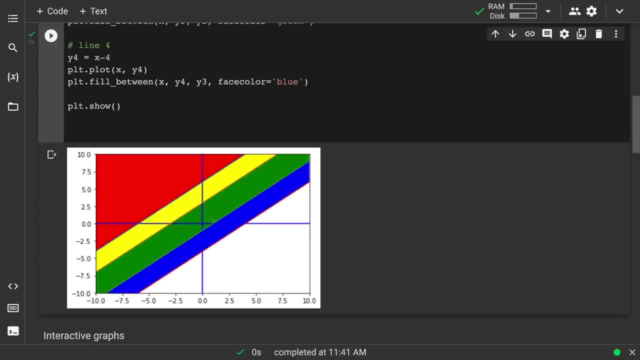 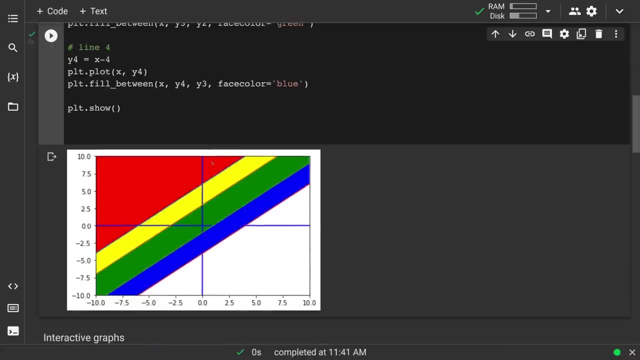 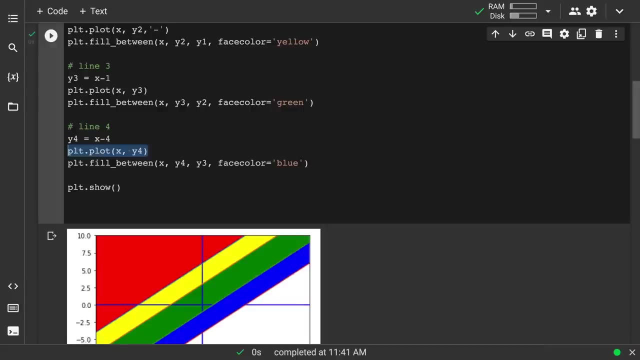 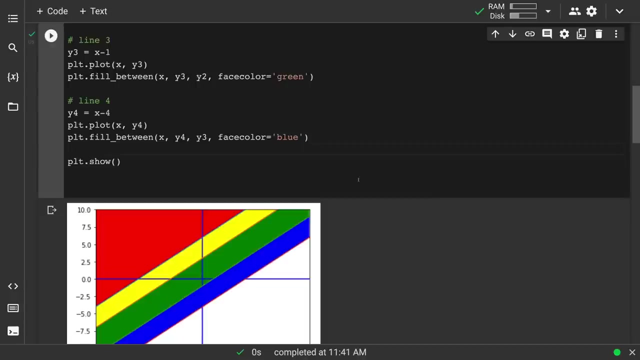 It's hard to see, It's a little bit. but you know, there we go. And because these, you know, with the shading sometimes you might not even need to plot the exact line. I mean, mathematically you might just be in the habit, hey, I want to also show that line. but the way it shows up on the graph you know it's not. you see the dividing line, you know it's nice. but sometimes you might say, oh okay, if I'm making some sort of art, sometimes I might not want or need that extra line. 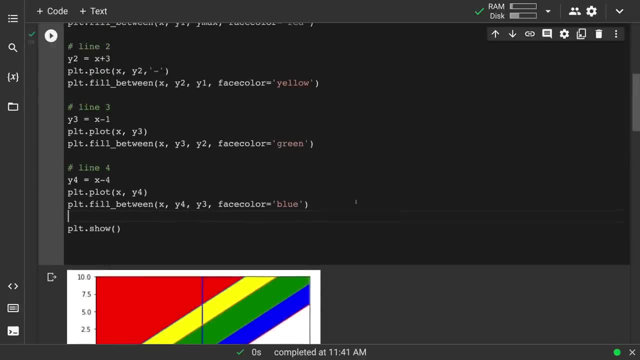 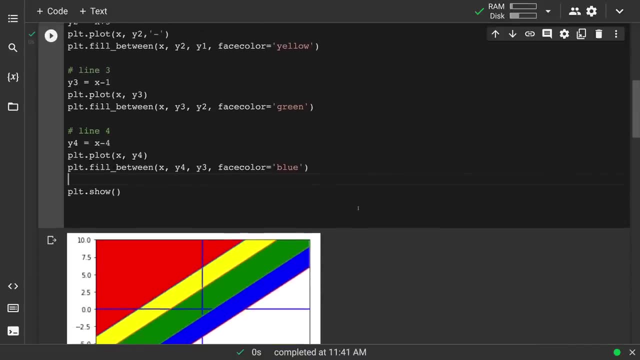 So there we go. So there's some different things you can do. you know draw lines, shade above and below, and you can be, you can get creative with this and make all sorts of all sorts of things. And this is essentially. you know what vector graphics are. you know not you know defining each individual pixel, but defining the lines that you draw based on equations. 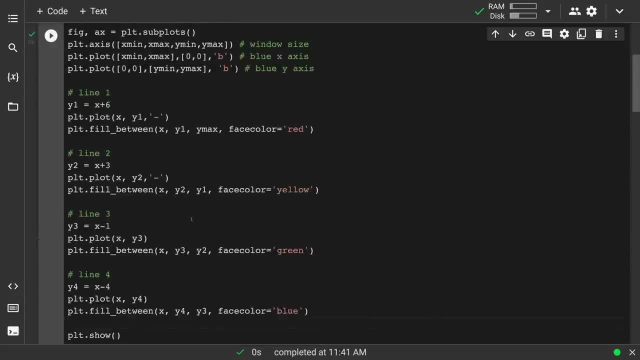 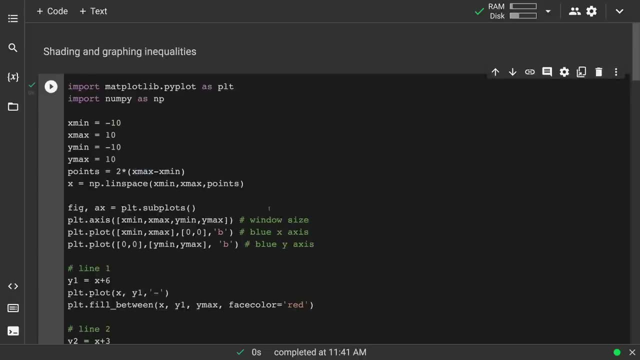 And then that way you can scale things. because Let's say, I wanted to scale that If I just changed the dimensions of my graph, I could scale this line with the same code and the same equations. So that's the advantage of vector graphics. 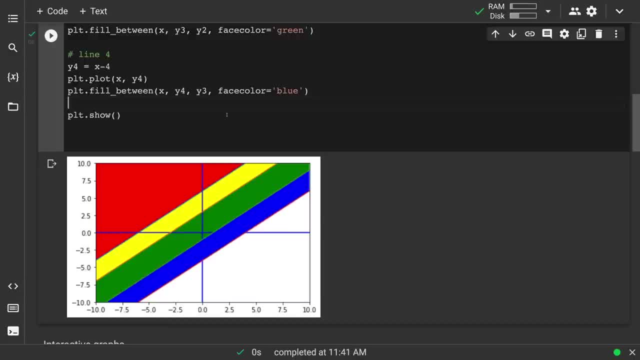 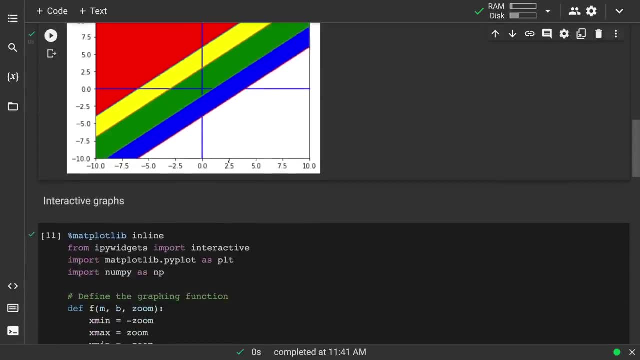 You can make larger things, but with not much bigger file size, because it's all defined on equations anyway. So there we go, Some, some cool things. you can do with that. Other cool things: You can create an interactive graph, All right. 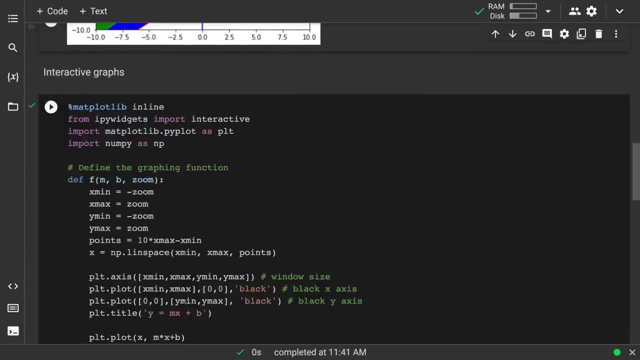 And with interactive, interactive- We're going to set up some sliders. This one's called interactive. If you might come across some Python code that defines sliders, it actually uses the word slider, that you know. that works too. But here's what we're going to import. 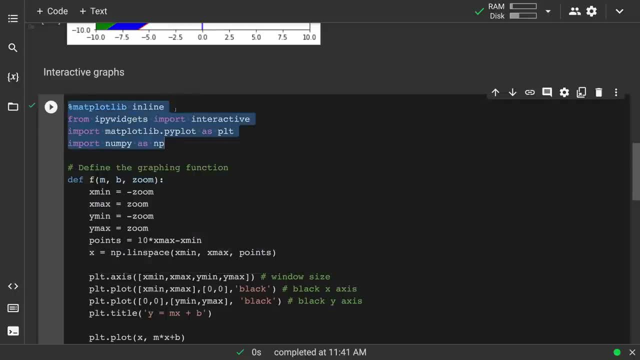 There we go In line, And the inline part is going to get us to be able to adjust these sliders and see the effect on the graph right away. So there we go, And then this interactive widget. So I'm going to define. 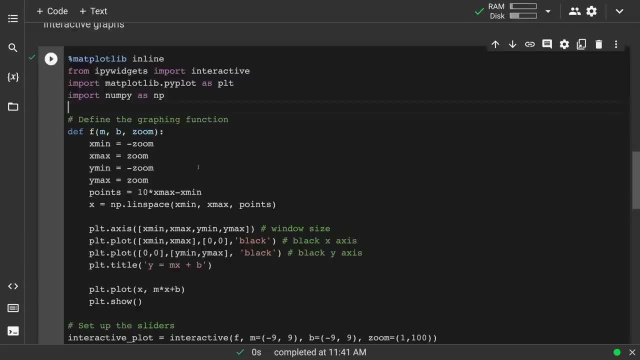 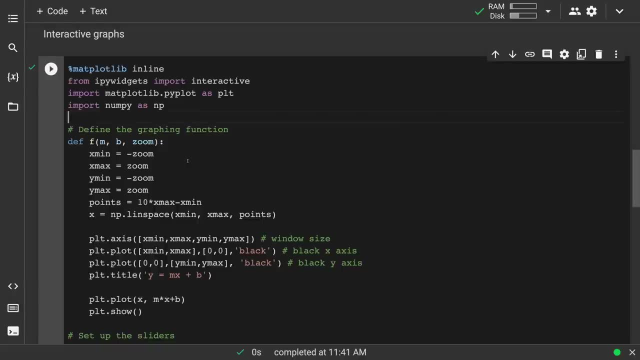 All, All the graphing notice is going to happen within this function. So I'm going to define this function. So, Again, I made it a simple slope intercept. So I'm going to define the function of MB, And then I put another variable for zoom. 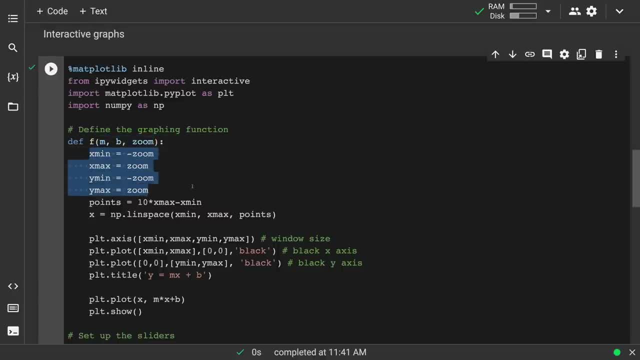 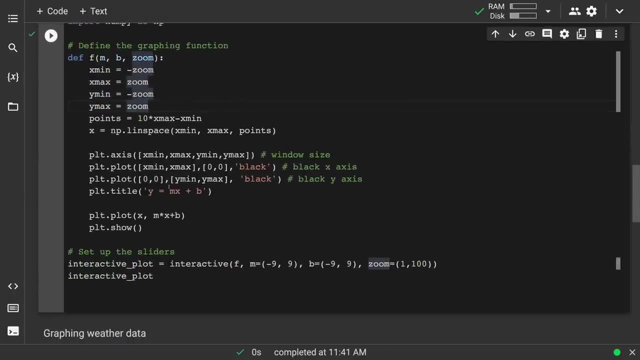 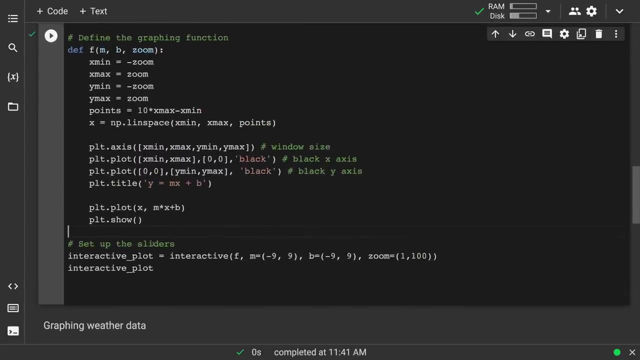 So notice, all of your dimensions here are based on that variable for zoom. And then we still have the points And the plot. that's my Y value, MX plus B. So now this function takes these inputs And here's the slider. 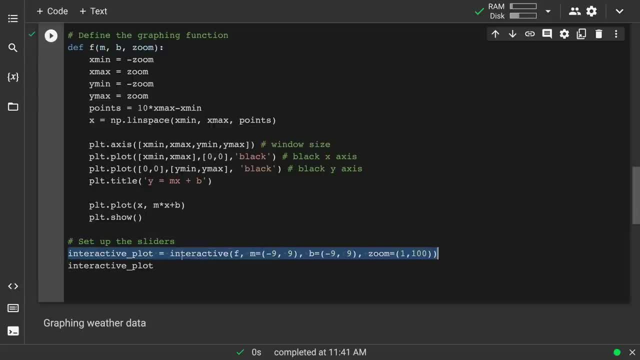 It's really the most of it is right here on this line. So interactive plot: Now I can make that whatever variable I want. I just decided to call it that and interactive Open parenthesis. So the first thing is, what function am I going to run? 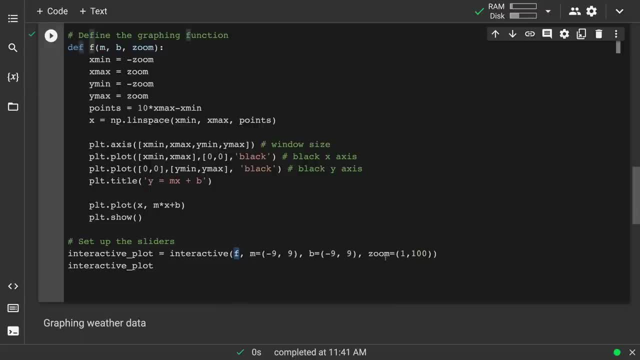 And I made it F. and the main reason I made it F is of the line. This line of code was not that long. but there you go. What function am I going to run? And then let's define some ranges here: M will go from negative 99, B will go from negative 99 and zoom will go from one to a hundred. 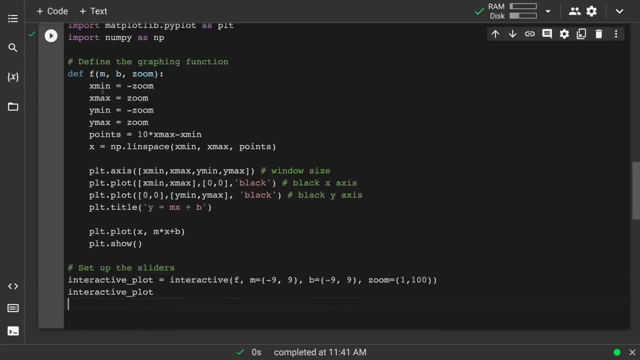 So notice the zoom. I could make it really small and X min max. you know I could zoom it all in. It's still going to be square. but I could zoom it really into just one in every direction, or I could zoom it out to a hundred and I could change that number as I see fit. 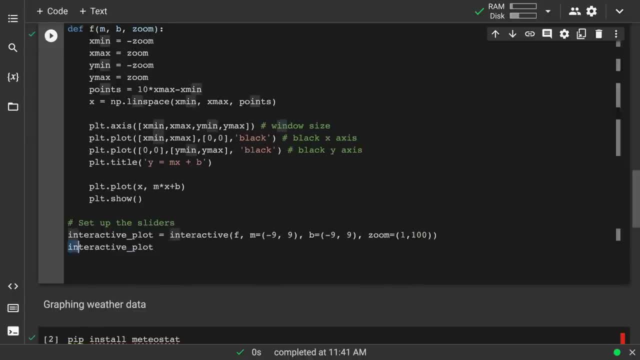 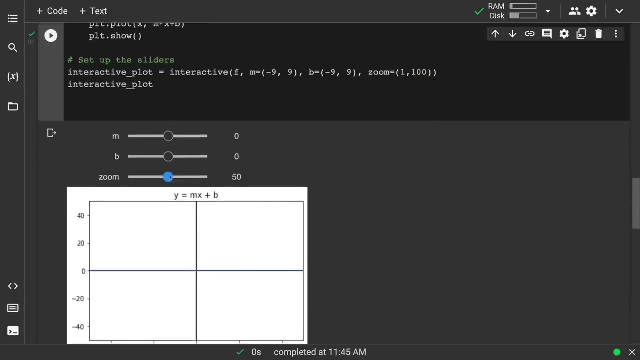 So there we go. So what we have is this: And when we run that interactive plot, it's going to take the input from the sliders and then run this function. So let's see how that works. So a lot of times the default puts everything right in the middle. 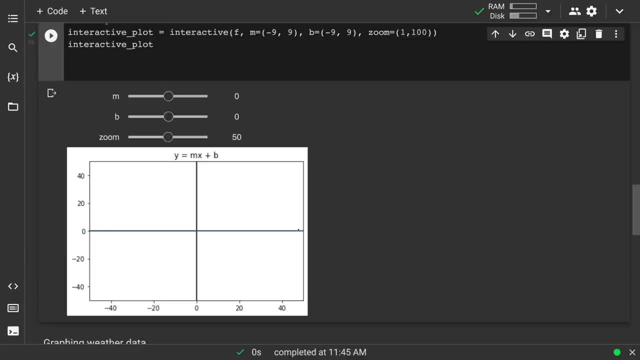 So my slope is zero and B is zero. So you might be able to see that the axis is black, but this line, this blue line, is on there because it's a slope of zero, zero, What. what happens when I move that up? 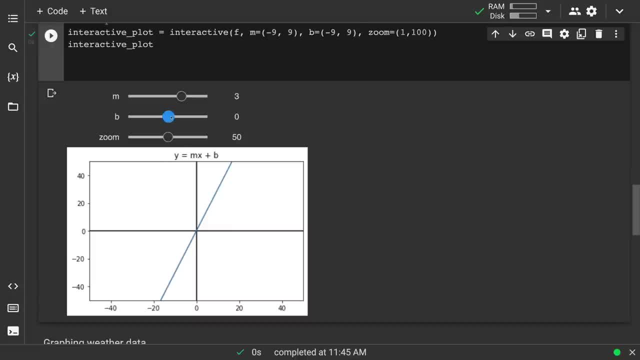 See, look at that Now I have a slope of three And as I move up B Then it crosses the Y axis at a different place. It begins right there. Now we see it starts right in the middle at 50. So I could bring this down and you see I can zoom in. pretty cool and see this is what I zoom. 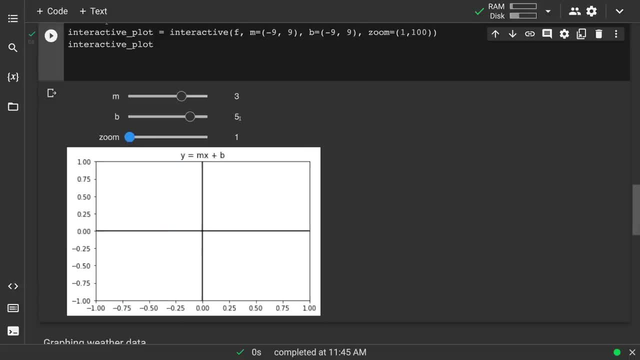 If I'm so zoomed in one every direction. notice B was five, So that's off the graph. now I'd have to move that back. Now you start seeing it on the graph, And these are some cool things you can do with your graph. 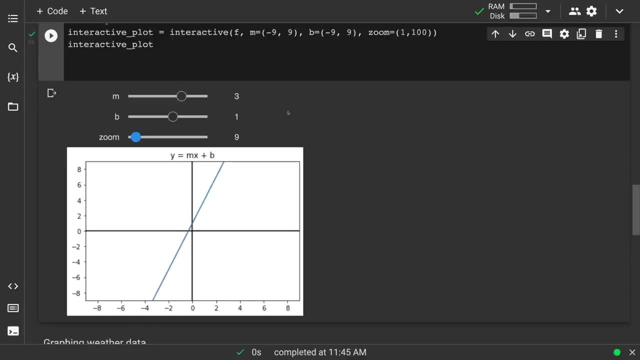 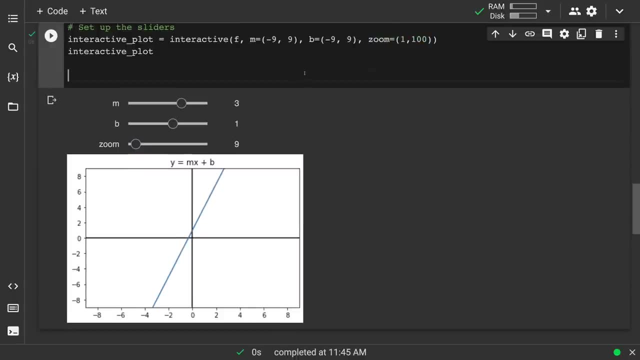 You can add this interactive, even if you- you know you're graphing all kinds of things- You just want to change the zoom. This is a nice way to zoom And you know you might see some things on other calculators where you can zoom. and here's how you can write the code. 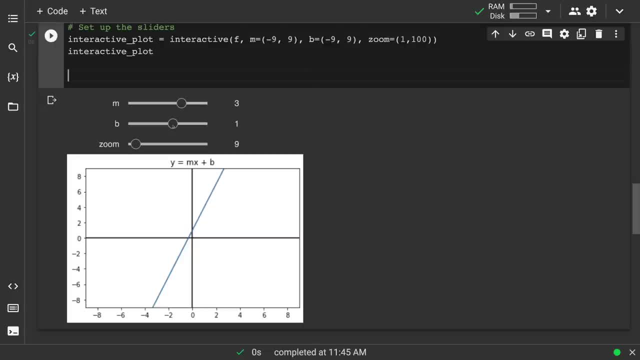 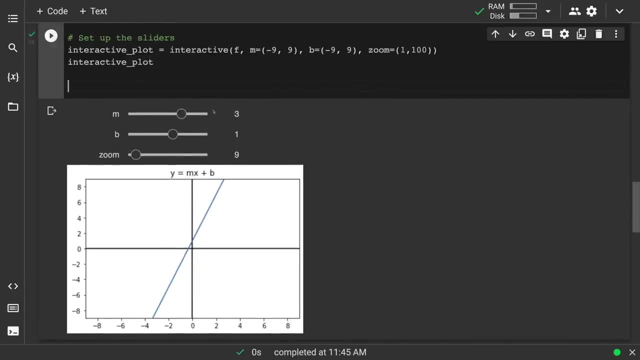 You can have your own graph that zooms in and out and you can adjust some other things. So there we go, Some cool, some cool things you can do. And I just want to, you know it's, it's a good way to illustrate, you know, slope and intercept as they change. 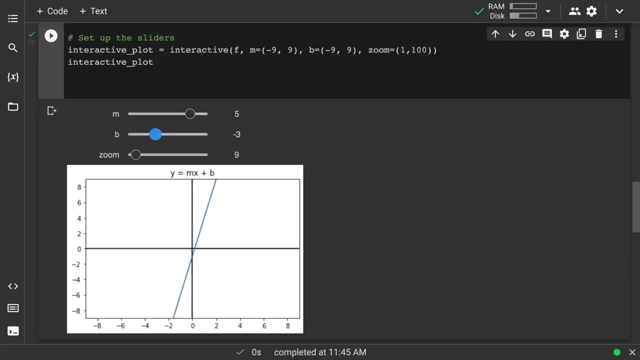 How does the graph change, You say, and then I can make B negative and therefore across the wax is down here and I can change the zoom, you know all the way. So now I'm really zoomed out and it it looks like this might even cross at zero- zero because it's so tiny. 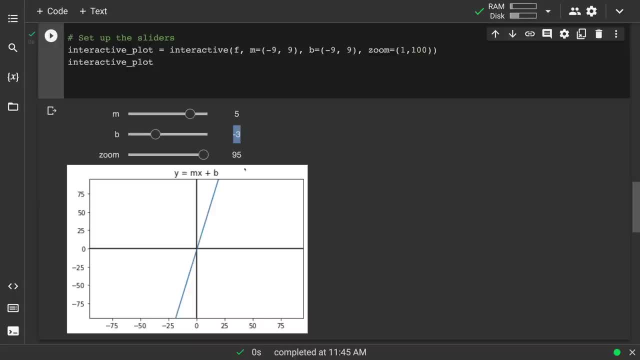 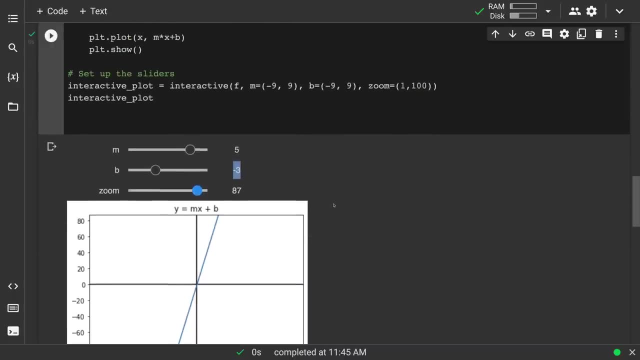 It Only crosses at negative three and my graph is so zoomed out. but there we go, Some interesting things you can do with zooming and you see the just. you make that interactive plot and then your function. all the graphing happens in that function. 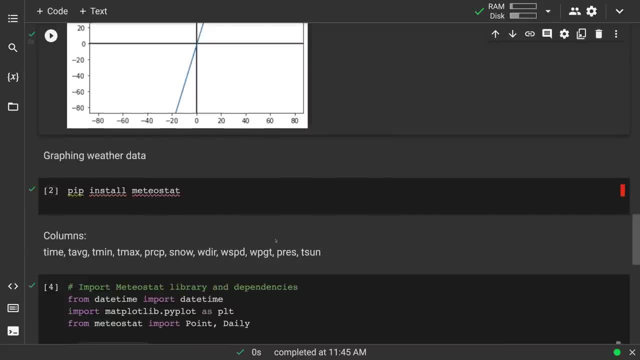 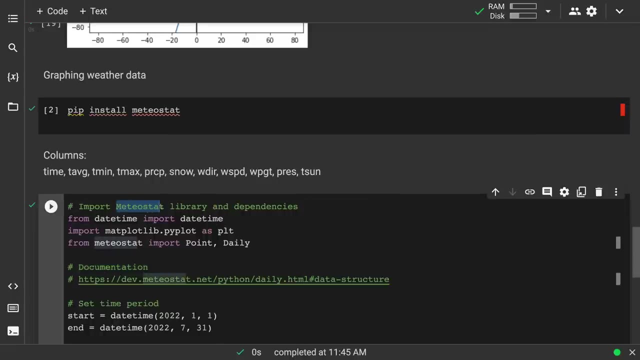 Okay. So here's another interesting way to graph. We can actually, because all this math is going to lead you to working with data science, So So let's just get a little taste of it here that somebody else created this library, this media stat library, for getting just some basic weather information. 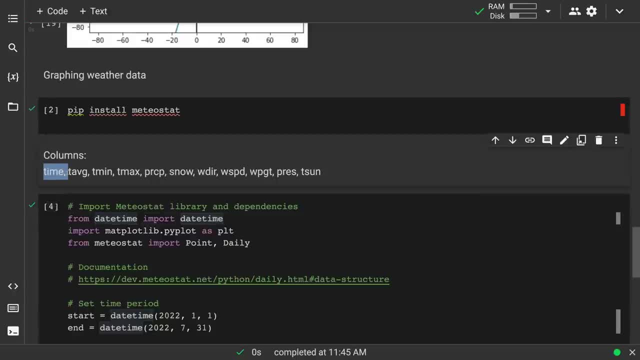 Here's- you know the weather information that that they take time. average temperature, minimum temperature, maximum temperature, precipitation, snow, wind direction, wind speed. This is the wind, The wind Gusts, The maximum wind gusts, air pressure and the amount of sun. 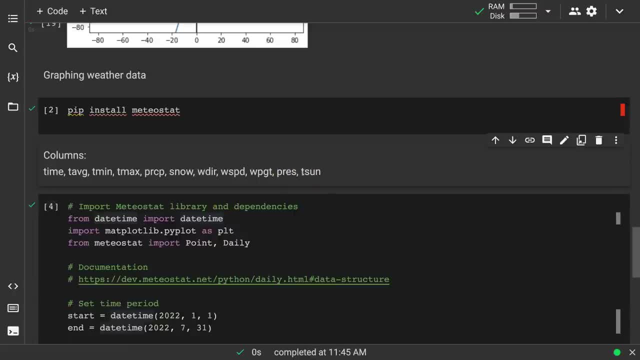 So there you go. planning setting up your solar panels. You can calculate the hours of sun at a particular place. Uh, planning to set up your um wind turbines, You can calculate wind speed at different places. and Here's how this works. 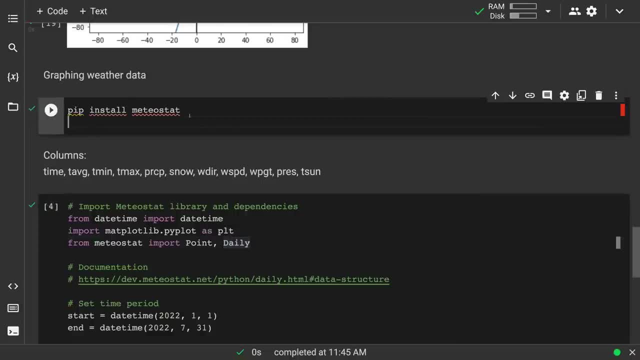 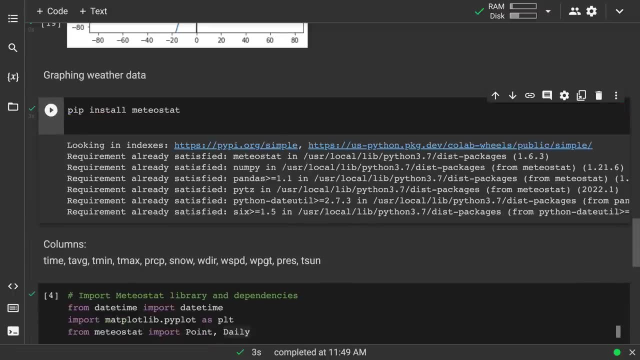 This one. you do need to install this, And so we're going to run pipinstall And I just made that its own separate code block. And there we go. We just see that this stopped running and that installed this. So there's a lot of things already built. 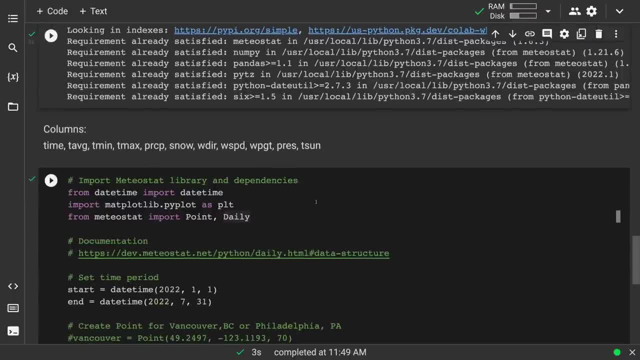 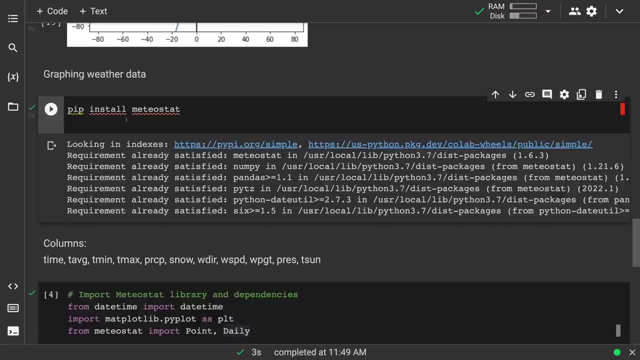 into Colab. You might have noticed we've imported some things but didn't need to install anything. This is a newer library and therefore it's not already built in. So some of those newer libraries, the install, I mean it's really pretty straightforward. pip install video stat. 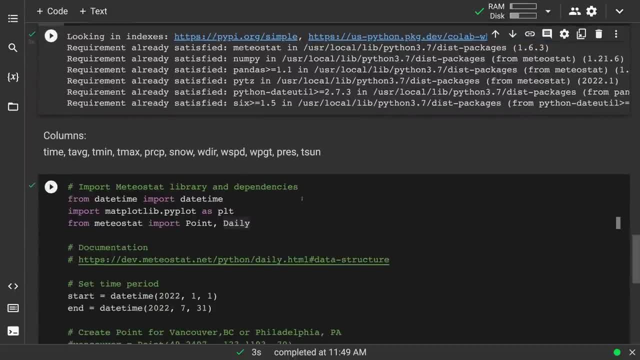 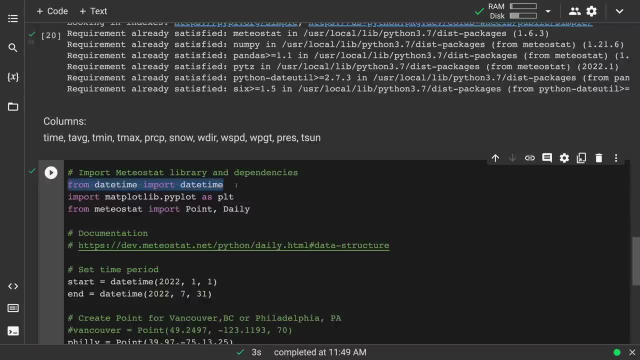 done So, install that library. Now we can import it. Date time: that was already a Python library, but we just do need to import that. And then now we still need to import this because we're going to plot this data, So that's why we import that. 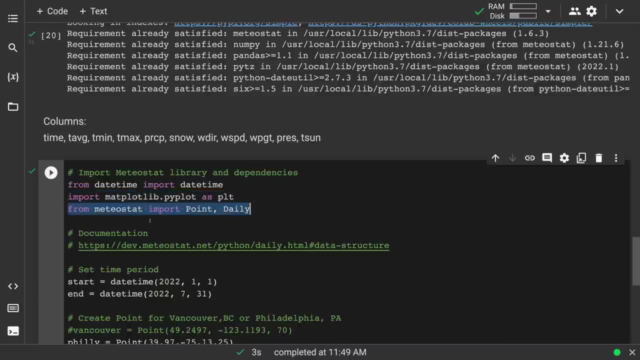 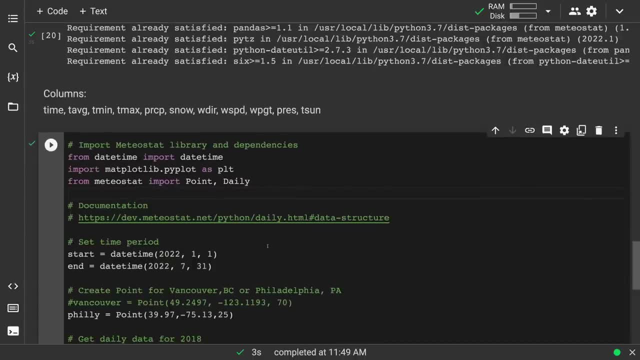 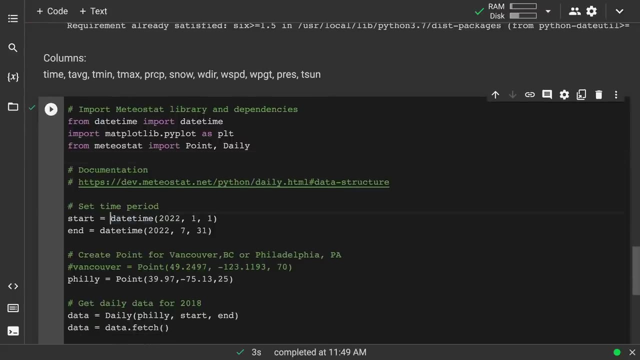 And then the install enabled us to do this: import these. I've included the link here for all the documentation. All right, so here's how it works. Start: we'll define these variables and they take this date, time, year, month day. year, month day. 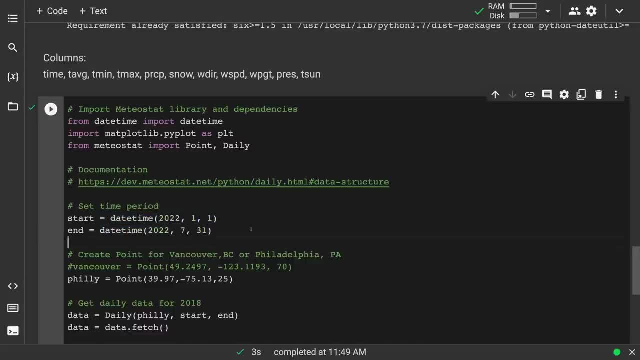 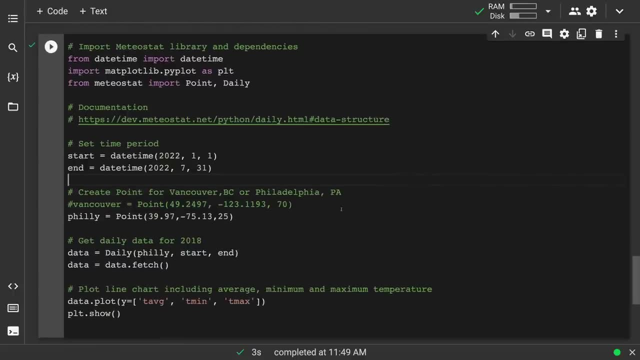 so I decided, well, let's do like the first half of 2022.. And so we have created a point. Now, the point you create this is latitude and longitude, So they don't have really built in like type in the name of a city. You want to have an idea. 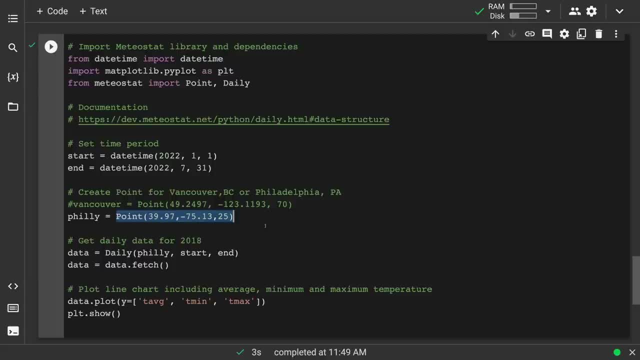 like you know where you live. you can find it like an exact latitude and longitude of where you are. You can find latitude and longitude. you know somewhere. you know if you want a particular city somewhere in the city. So the example that you might see if you look up, look this up. 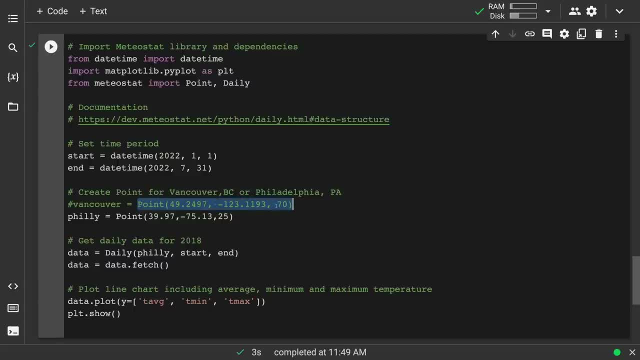 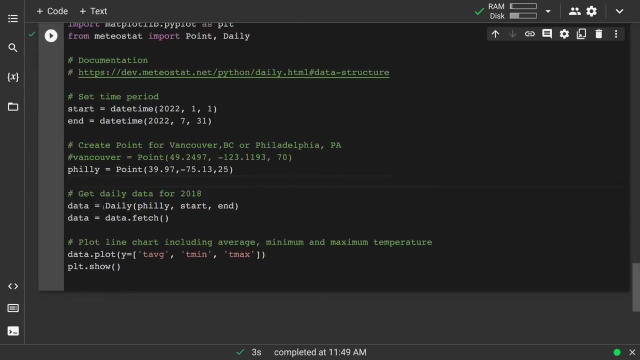 you know, somebody did this for British Columbia, So I changed it and did this for Philadelphia. So there we go. So here's a point in the middle of the city And we can just get the data here. So from that point, so 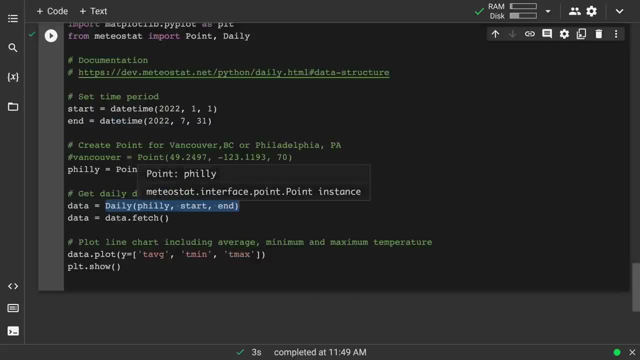 there we go, data daily. And then there's my data point, Philly, and start and end. So there we go. So we have this: you know start date, end date, location, and then collect the data. It seems like this would overwrite it, But this does work. using the same variable, data equals. 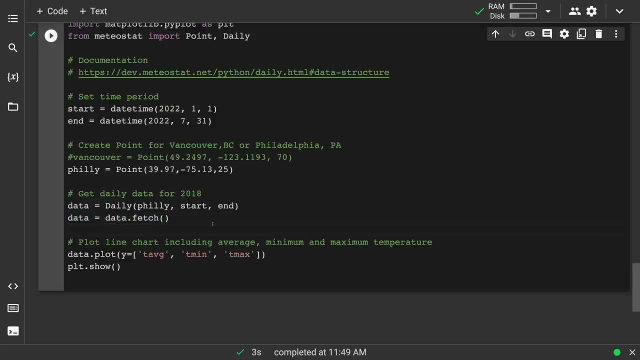 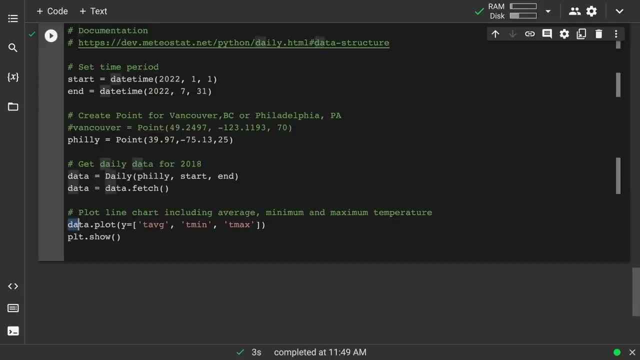 let's just plot the average temperature. So notice it looks very similar data dot plot. And then down here we have PLT dot show, But there's nothing else we need to do it. actually all the rest of it, the dimensions and even some other things, the way it labels the graph. 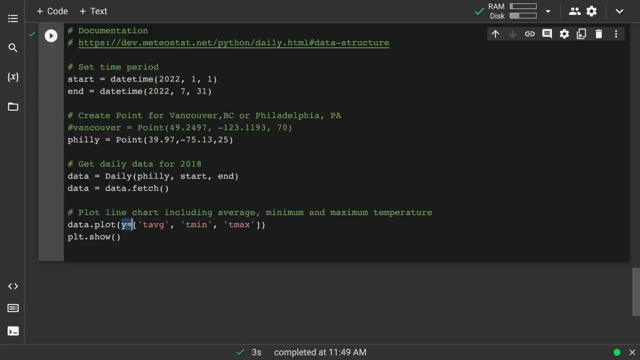 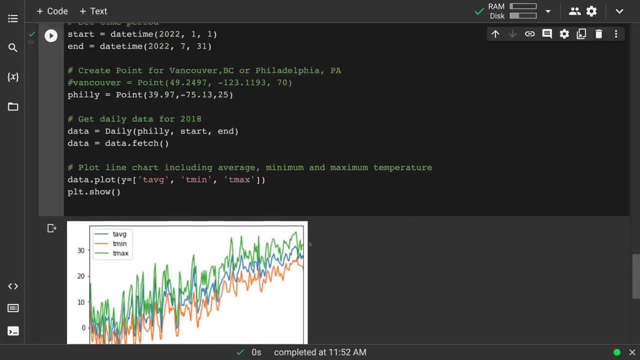 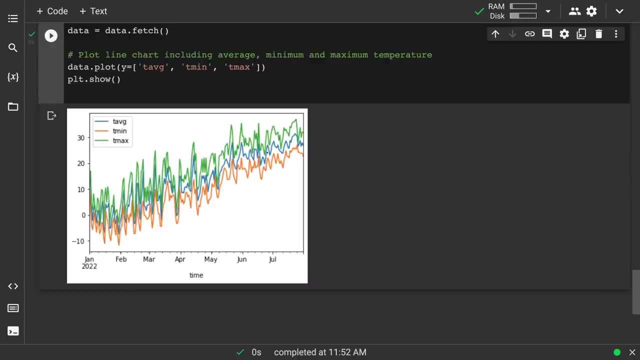 happen automatically. So there we go, we just have y equals and then we're gonna plot these three things. So when I run it, the average temperature, there you go. average min max. so all these things we know. in a previous video we were talking about you know how to create a legend. 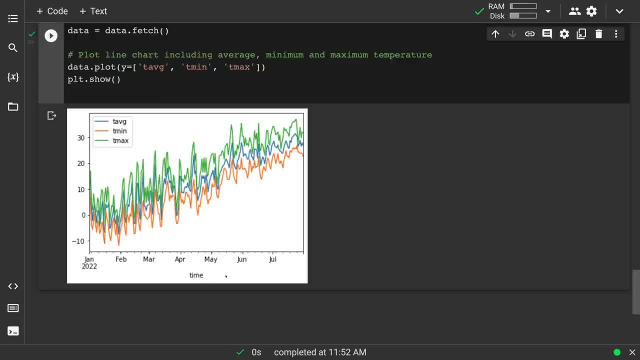 how to label the axis and everything. this already does all that for you and it'll just graph what you have here. all right, so there we go and notice the temperature is in Celsius. so there you go. if you're in Philly, you're like, hey, it hasn't been 30 degrees here in a long time. but yes, this is Celsius, so notice. 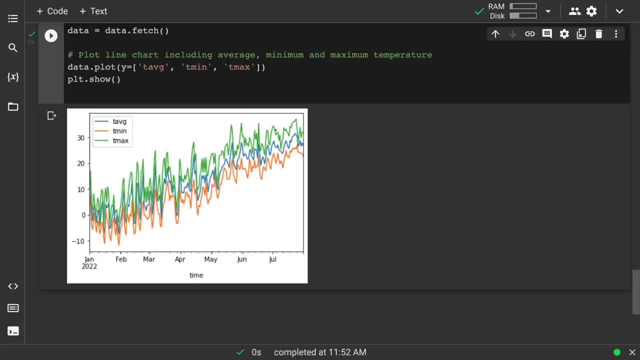 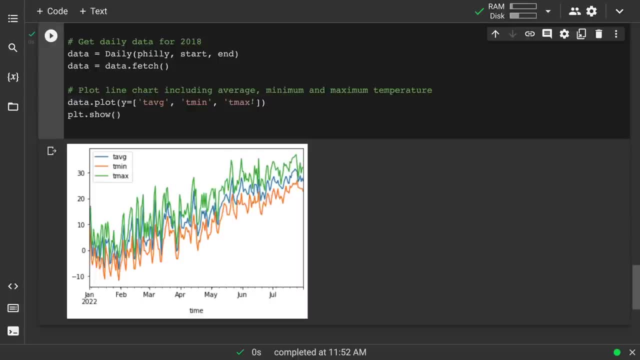 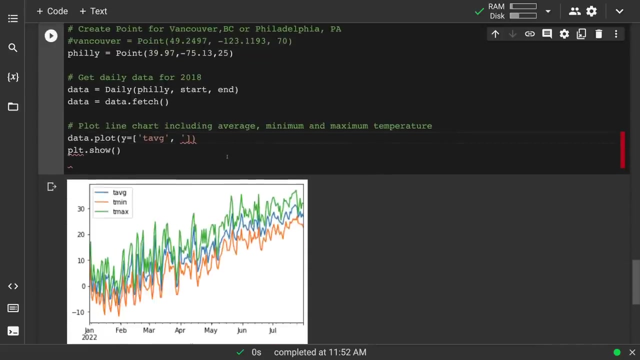 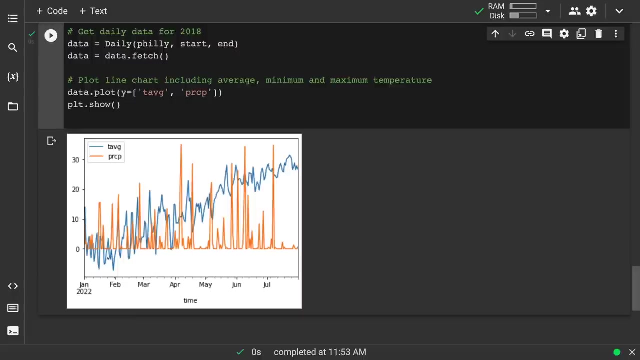 it's going way above that. yep, June, July, pretty hot, and then we can just change this, that we can have temperature average. maybe we'll keep that and maybe we'll do one of the other ones: precipitation, PRCP. there we go, so we'll graph this and we see so average. 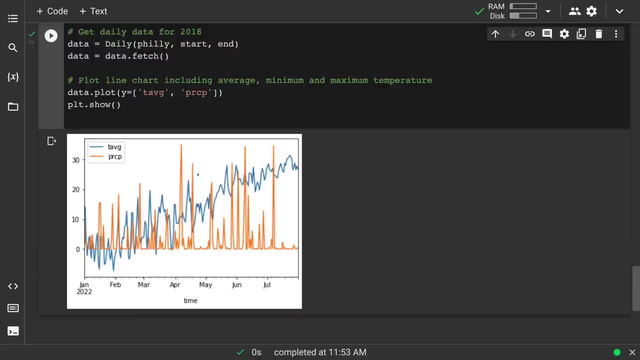 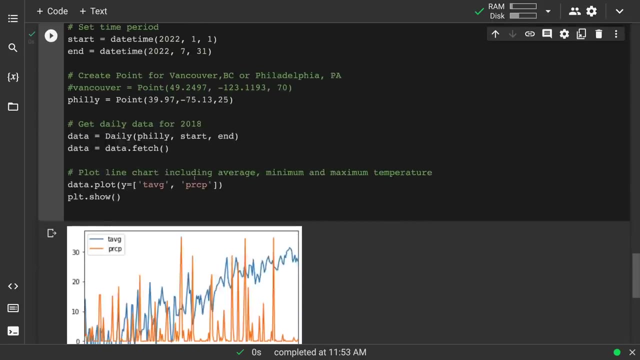 temperature and then precipitation: there we go pretty cool, and we can see that it's going to be a little bit lower than the average temperature. and then precipitation: there we go, pretty cool, and we can see. and of course, then you know, there there is another one here. snow, now what? 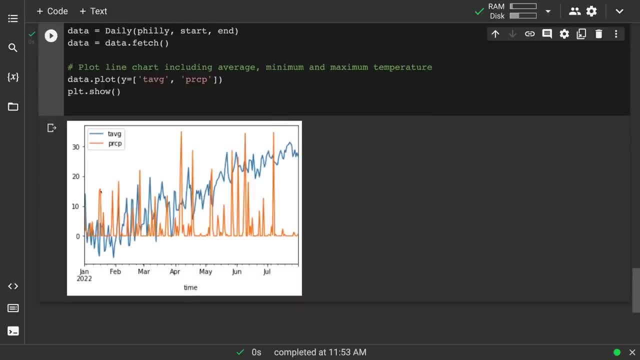 you can see is all right. if there's average temperature below zero and then precipitation, then you'd expect, hey, maybe there's going to be snow, but we can add that and you will see. so so we'll grading here that. there we go, there we get the prettyeni and that snow. 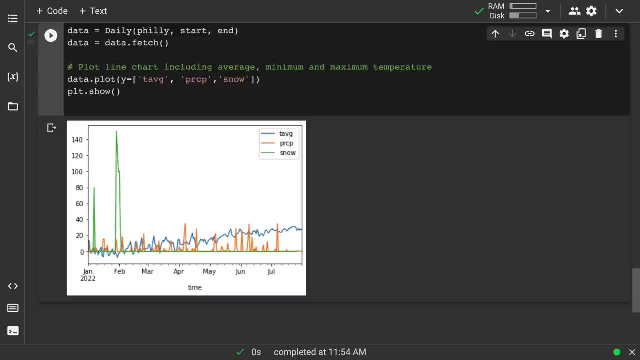 there, you'll see that right. there won't be on that, Mary O'Ne่el, and the snow is going to be the only temperature on the more. just The mother precipitation. there we go. snow isn't green and you'd think. look at that average precipitation. 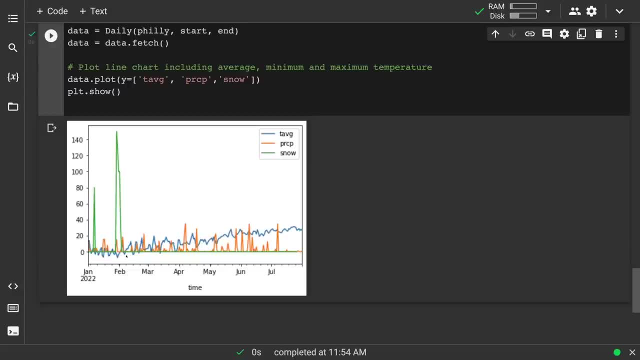 favourites in Europe, because number two, what uses precipitation is for- has means, though we've got a name of it's important, and בעhmenüse, and there precipitation and below average temperatures, but no snow precipitation, blow, average temperatures but no snow below zero temperatures, and it's kind of 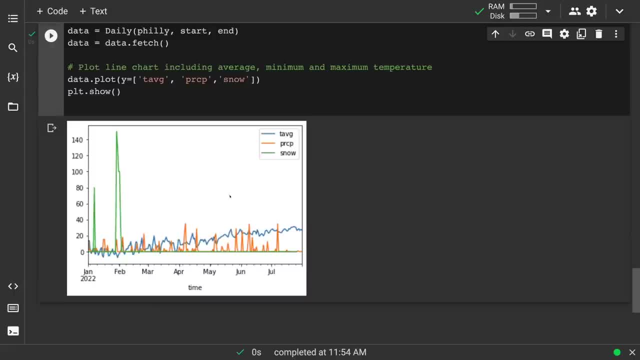 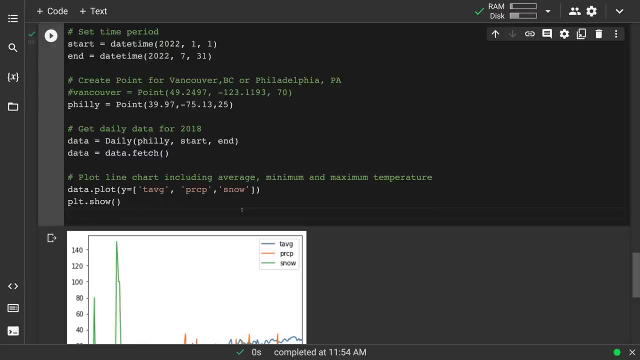 and there we go. That's it. So interesting things you can do. And you know, even, uh, we were talking about having this on your you know, having the collab app on your phone. you could have, um, you, you could have something you know related to uh, you know. 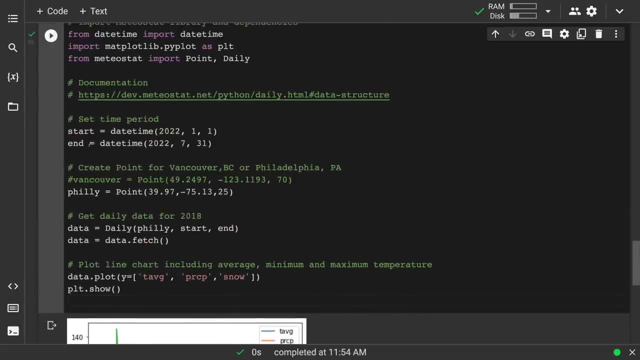 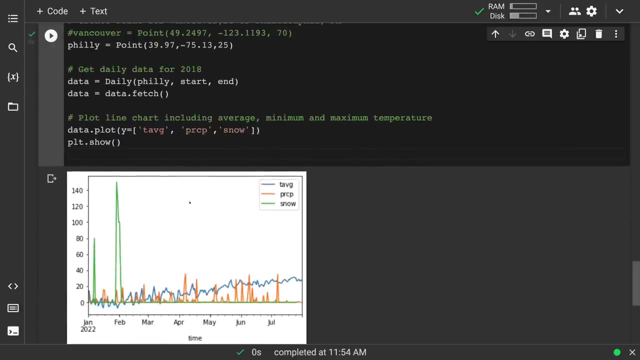 write, write another line in here to get you know, to get today's date or yesterday's date and sort, you know, use that as the end date. and you know, have your app and click on, click on something, run it and you know, see the historic temperatures, or snowfall, or wind. 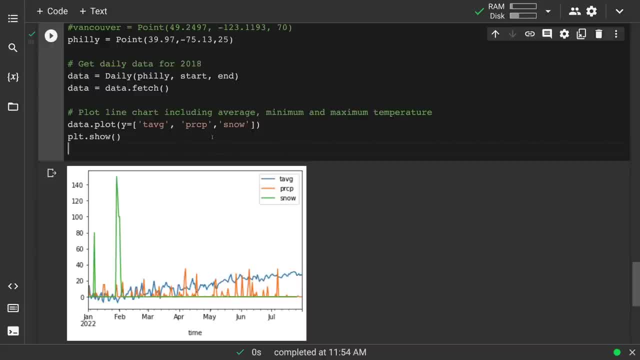 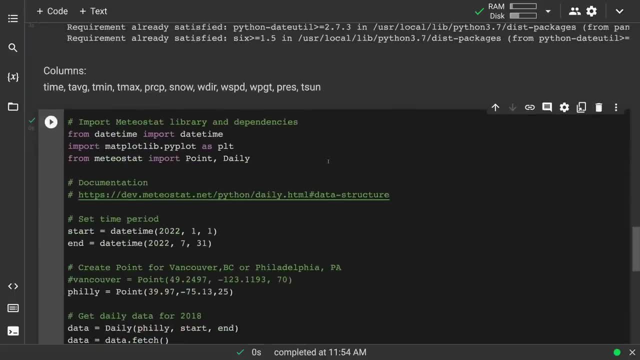 up till now. If that's interesting, you could do some other things with this. So just some good things we can do with graphing and, you see, just getting a little bit of taste to how. this is why Python is so good for data science, because a lot of people make these APIs. 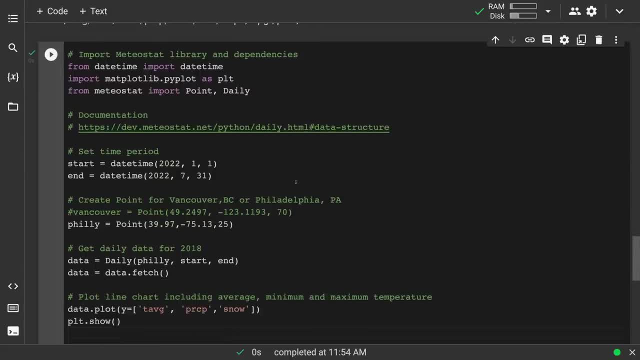 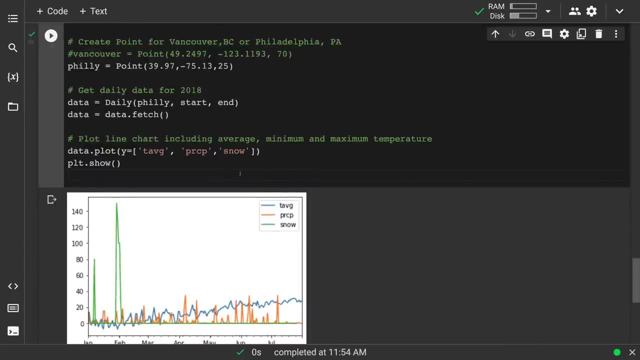 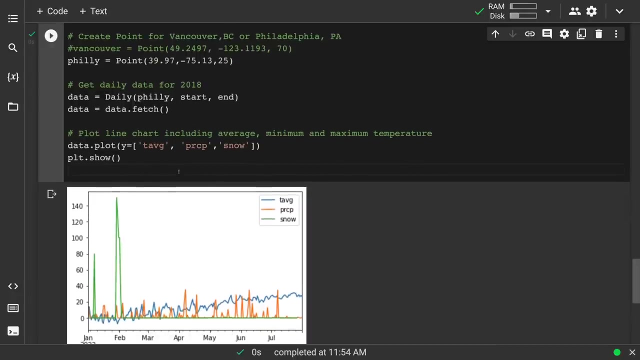 that you can just write a few lines of code and get the, get the data you need and automatically graph it. It's pretty powerful like that And you see the, the graphing that we end up doing is the same. you know, map, plot, library, So pretty good, Some some cool things you can do. 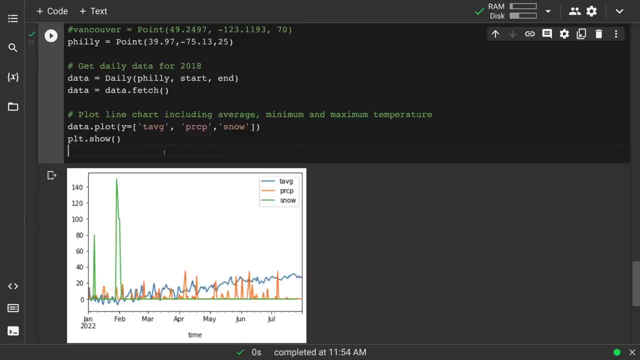 with graphing, and, uh, we'll continue on the theme that you know. next, we'll look at solving equations and graphing. you know all together Which ends up being tricky, but we'll show you how to do it, Okay. So, yeah, take a look at this. 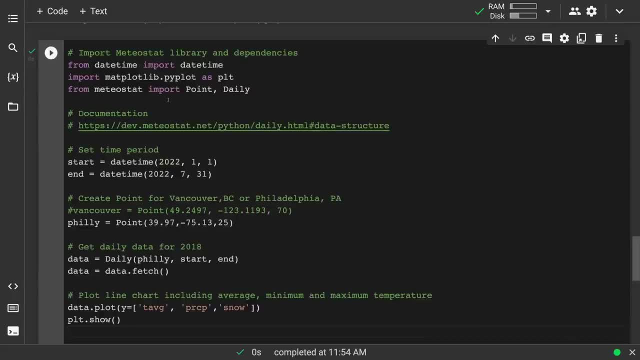 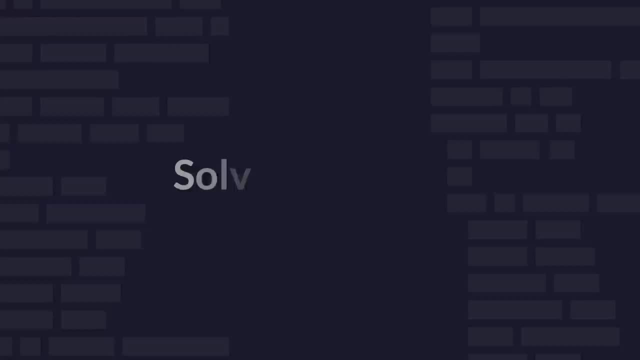 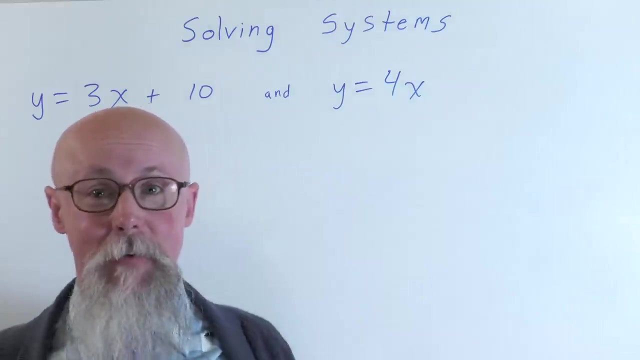 tinker with it. you know, set up some. you know some. you know weather, weather weather report code for yourself. All right, Now we're going to look at how to solve a system of equations even without the graph. 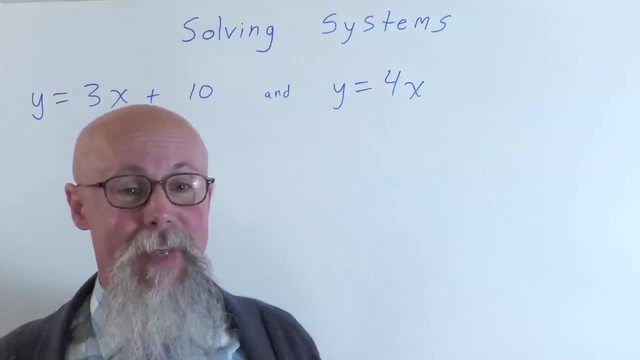 And you can still picture the graph, The idea that that's, that's what this is. These are two systems of equate, These are two equations, two functions that you could graph, but I don't need to see the graph to get the solution, And sometimes for solutions that 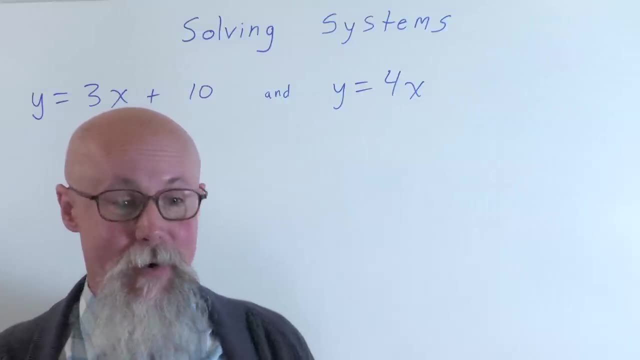 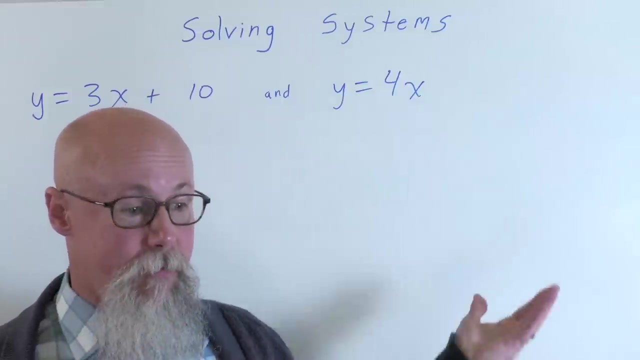 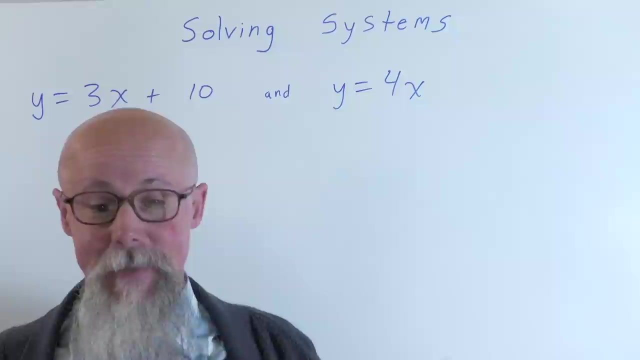 it might not be easy to see on a graph, then you know, maybe it's, you know, not in a nice integer solving this. this is going to work each time. So we're going to look at how to do this just on paper or on the board, And then we'll look at the code on how to do this um and set it up. 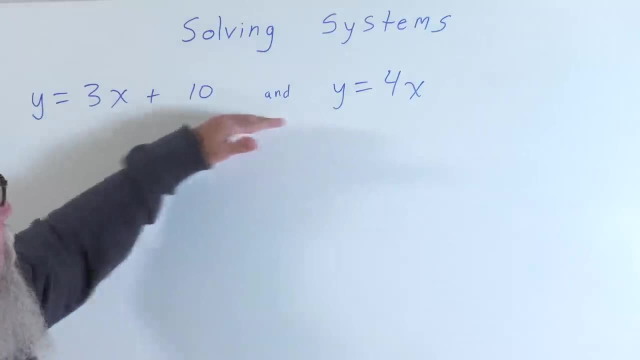 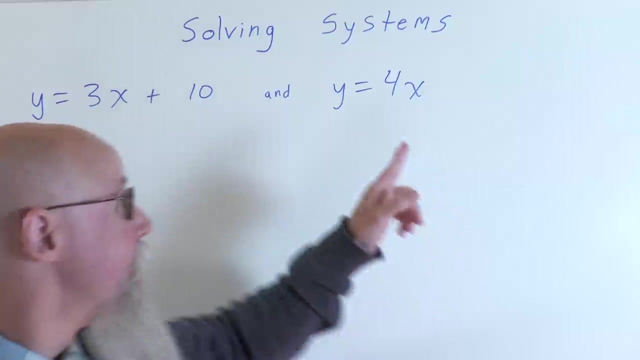 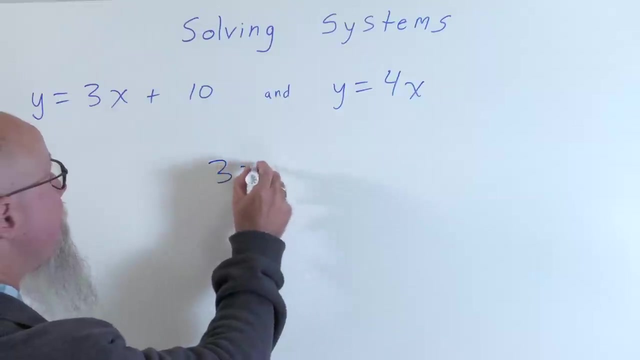 and just change the equation. So if I have these two equations, one of the ways to solve this- and this is some version of substitution- is if we notice: if this equals Y and this equals Y, then they can equal each other. Then three X plus 10 equals four X. 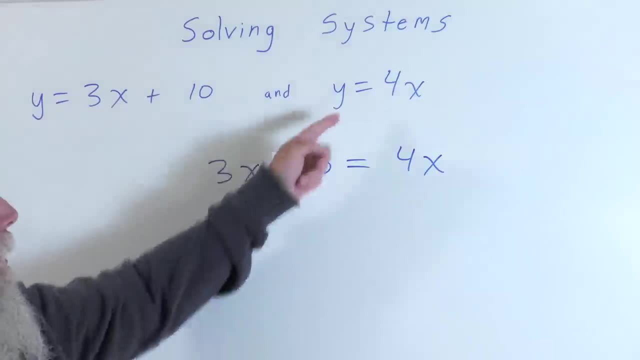 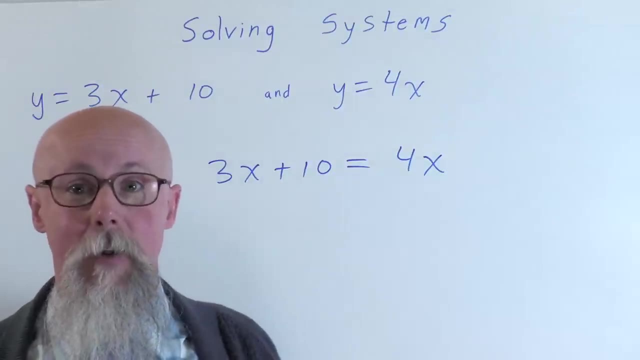 So we see that if that equals Y and that equals Y, then these must equal each other. Three X plus 10 equals four X. Three X plus 10 equals four X, And that's a little bit of the logic that's inherent in in all of math. 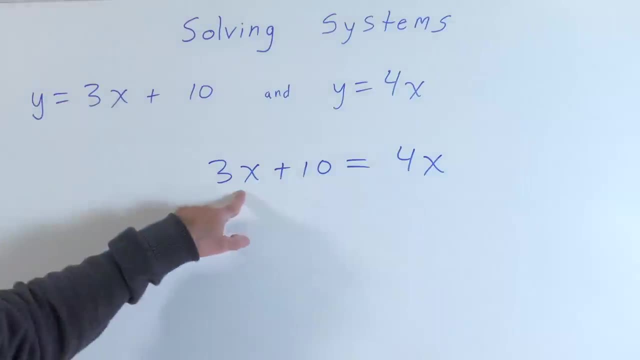 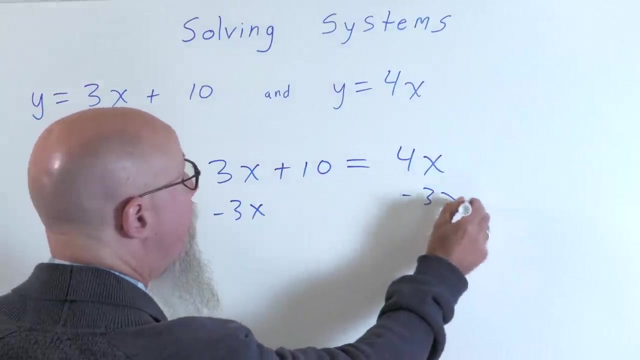 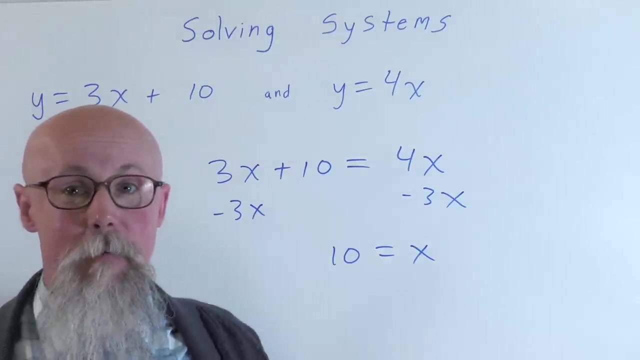 So now we can solve these. What can I do to solve for X? I can subtract three X from both sides And then I get 10 equals X. Now, once I solve that, X is 10, well, I want a point. So that's my X value. I need my Y value and I can plug this in. 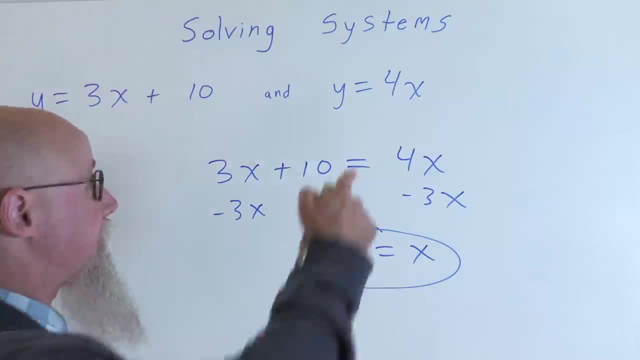 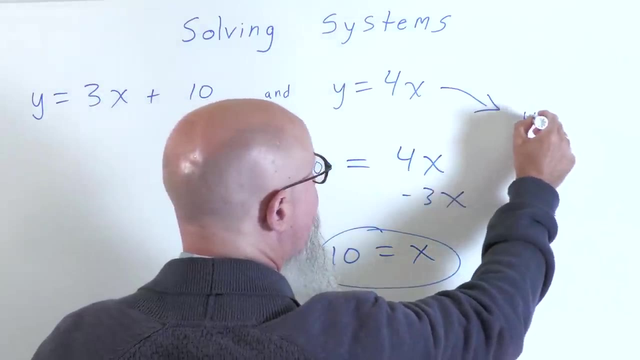 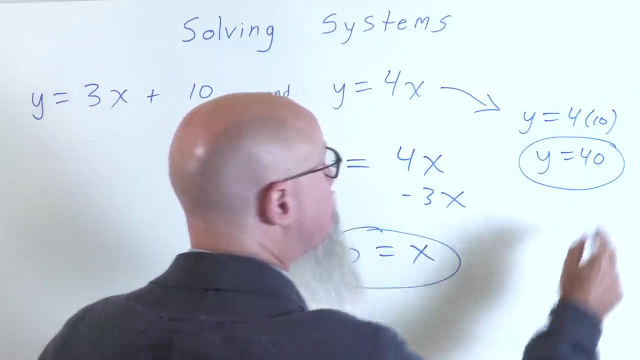 to either equation. So I would take this, and let's say I want to plug it into here- So Y equals four X, then I could take that, and Y equals four times 10. And that gives me Y equals 40. And then that's how we would get the solution. We can set these equal to each other and then 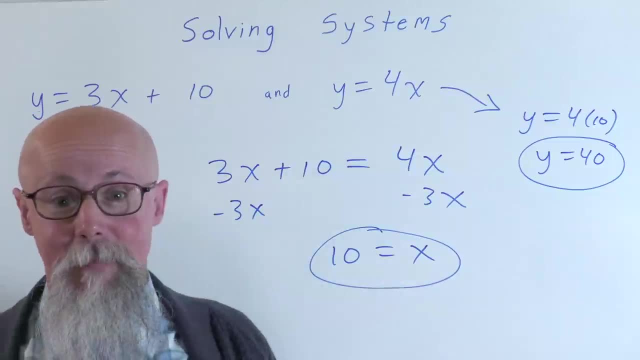 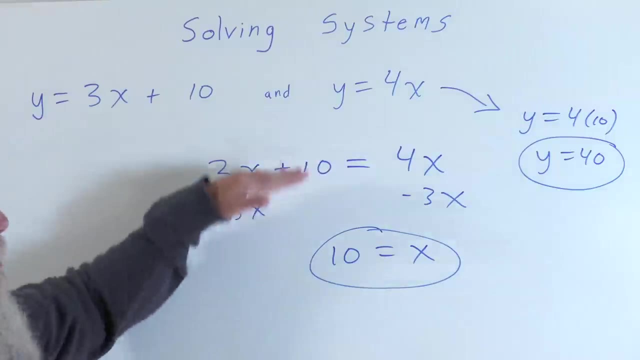 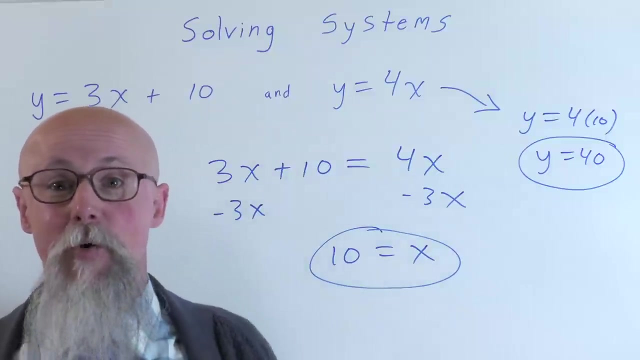 solve. solve usually for X, um and then plug that in Either one of those and then get our Y value. Now, this is very similar to how this is going to work out in the code. One of the things that makes uh sim, the SimPy library and solving this. 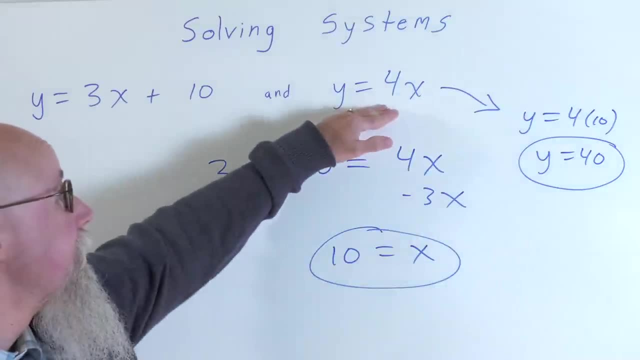 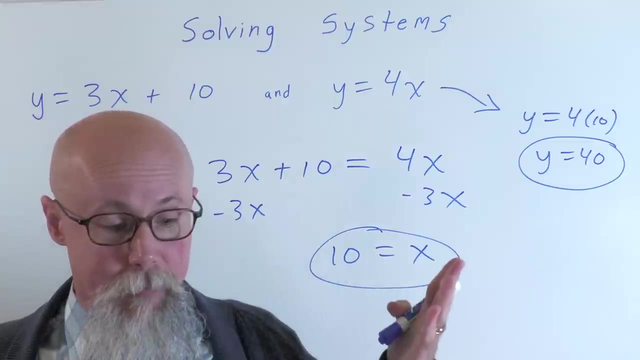 with Python a little bit better, is? this works out nicely when they're equal to Y, And you know that looks, but if I had equations, um, that were not equal to Y or something like that, um, with the Python code, what I would do. 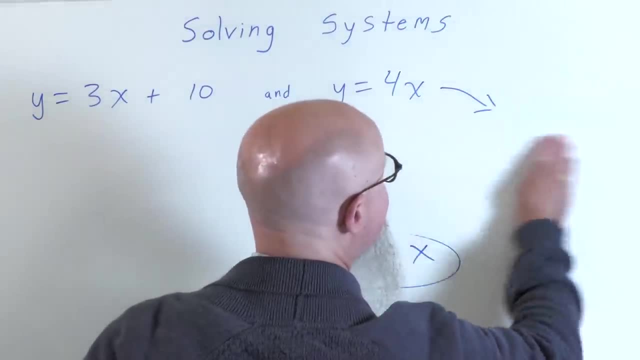 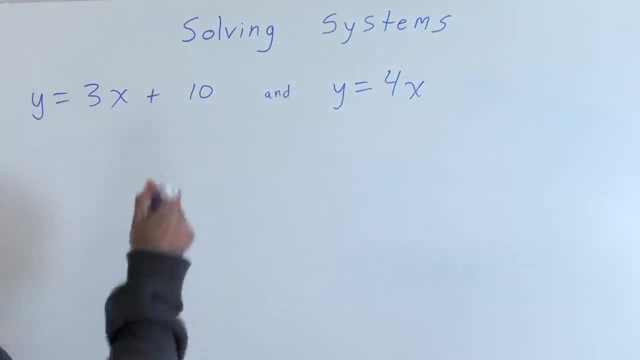 and we would do the same thing with this is the idea that I would make. I would want each of these equal to zero, So I would end up subtracting Y here, So I would get you know three X plus 10, and I subtract Y from both sides equals zero, And that's the version I'm going to want this in. 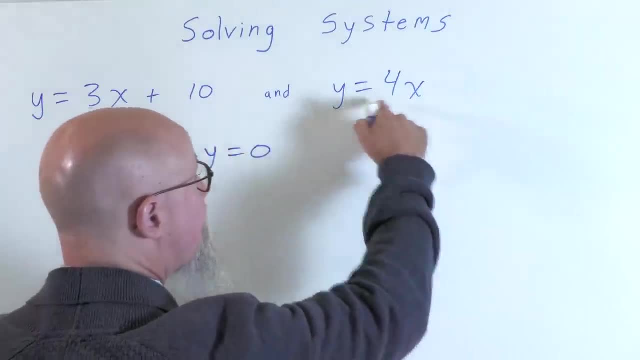 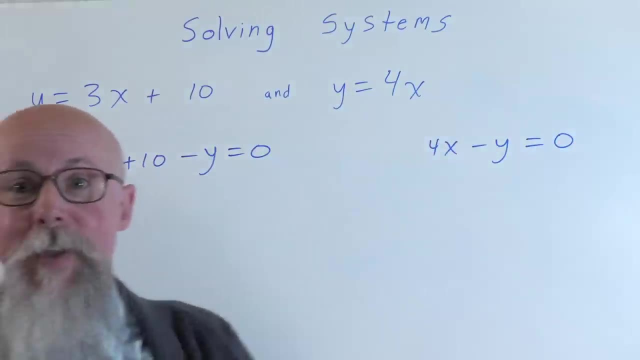 when I solve it with the code. And then the same thing here. you know, four X minus Y equals zero, And then with each of them set equal to zero, then you will. we'll see how that that plays out using the SimPy library, but that's. 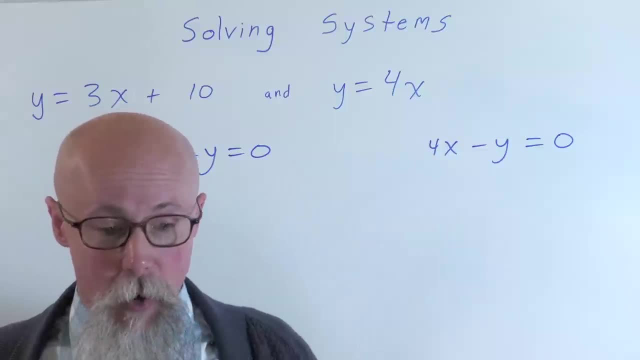 that's kind of the method that Python uses to solve. So one of the advantages of this is they they could be in whatever form they want. whatever you have on the other side of the equal sign, just subtract it over And then now you have two equations equal to zero and you can solve it. 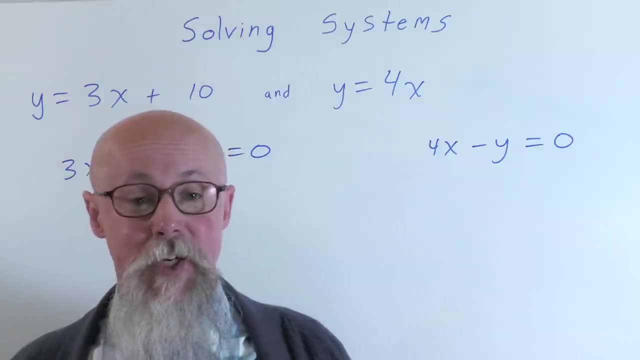 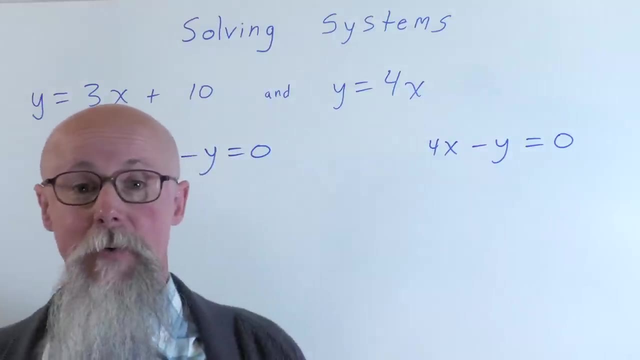 So you know, and there's many other ways to solve systems of equations, but that's kind of the couple of ways I want to show you. you know this, this type of factoring where you can set these equations equal to each other, solve for one variable and then get the other one, And then. 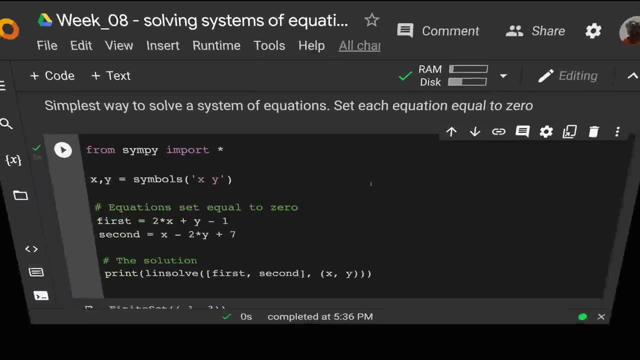 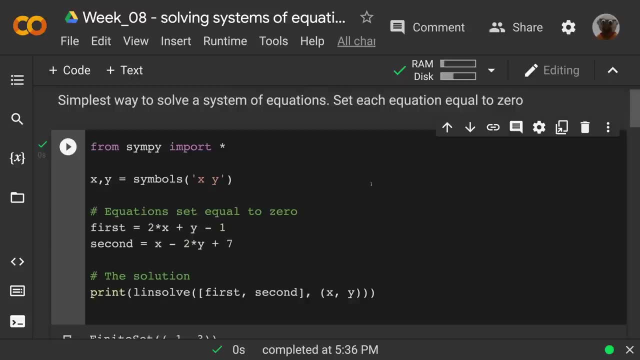 we'll take a look at it now. So let's take a look at the code. So let's start with the simplest way to solve a system of equations. Now, this is especially for linear equations. So you want to do that. The best way to do that is соответing this code out from your 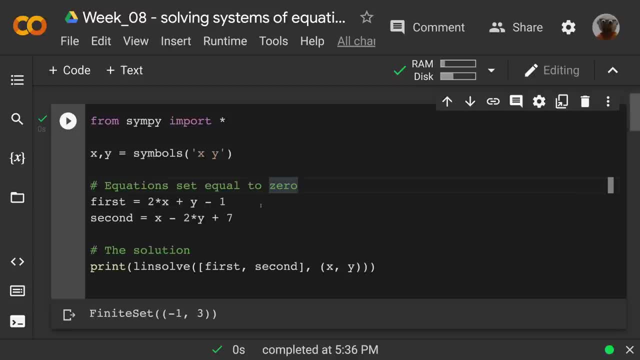 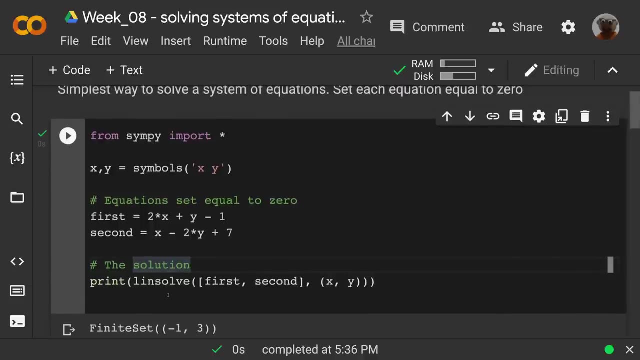 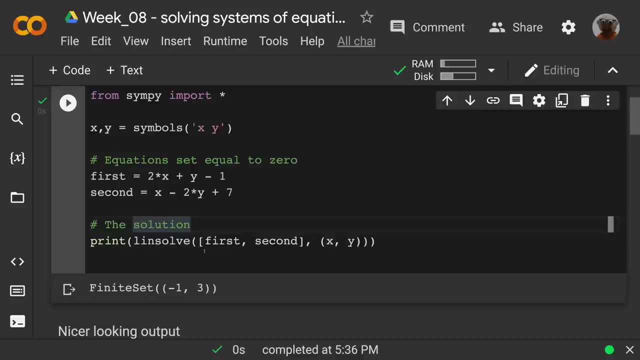 code. here we go now. here's the equation: set equal to zero. so first one here and second one here. then i just defined it as first and second and here's how we get the solution. so this is the lin solve, is the is the formula from simpi lin solve, and it takes- notice the extra brackets, first comma, second. so 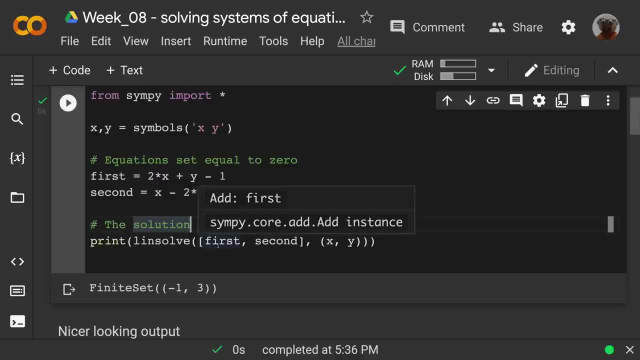 it takes this as essentially an array of two different equations. and then the next argument, comma x, y, in an additional parentheses. so it's using these symbols. so linear, solve these two equations, because if they're each set equal to zero, we can set them equal to each other. 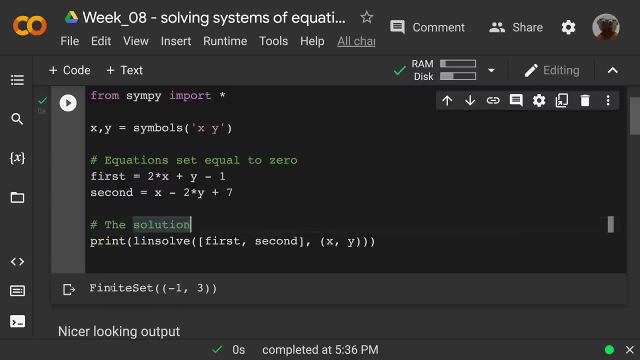 and use these symbols and when you run this- i already ran it- we see it comes out as a finite set. now again, the simplest way is: there we go, we set these and here's the one line that puts it all together. you can just change. you know, change these two equations and run it, and you know, you see your. 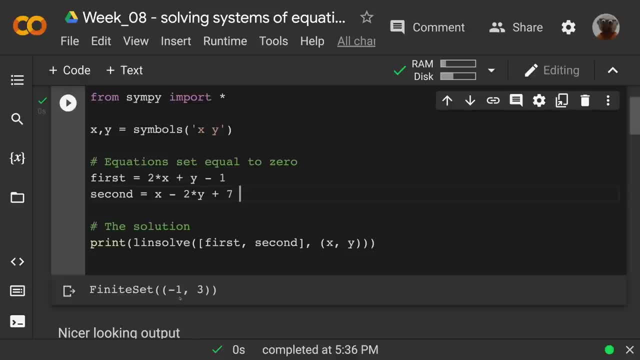 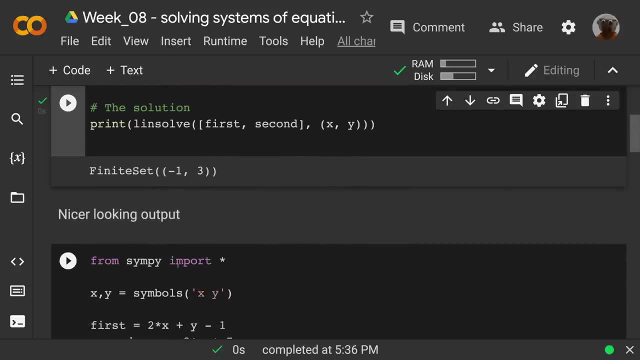 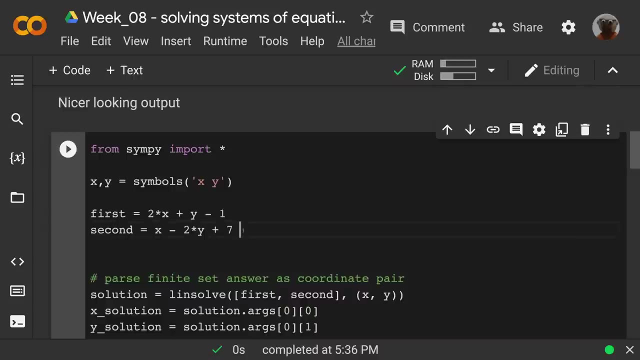 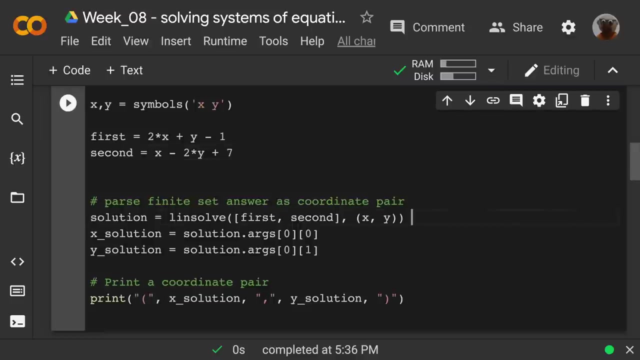 answer. it's pretty clear. it's a finite set. x is negative, one, y is three, supposing. i want it to look a little bit nicer, so still importing everything from simpi and these symbols still have the same, i'm going to use the same equations first and second. now here, where i have. 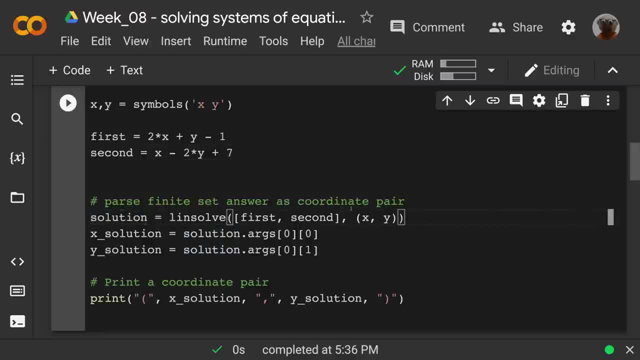 this solution here. that's the same line, but now i know that this solution variable is going to be a finite set, but there's things i can do with that. so i'm going to create another variable x solution here and i'm going to take this solution, dot args, zero, zero, and i'm going to 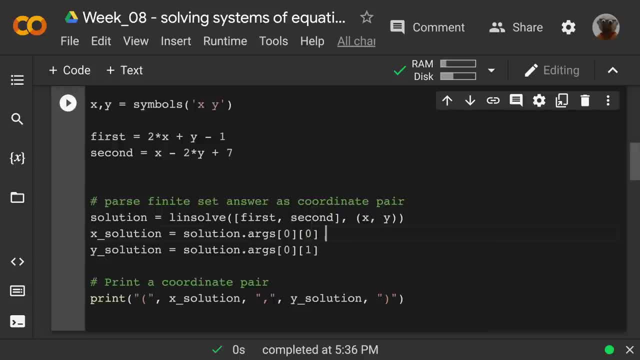 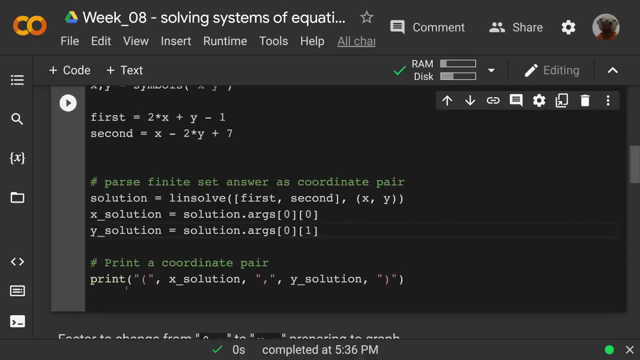 take this solution: dot args zero. notice it behind the scenes: it's a two-dimensional array. so i want the first thing and then the y solution, also a two-dimensional array solution, dot args zero one. so, having this, i can print a coordinate pair. so there you all. print the parentheses. x solution. 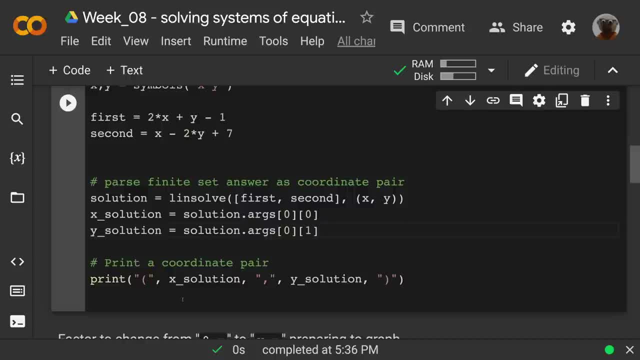 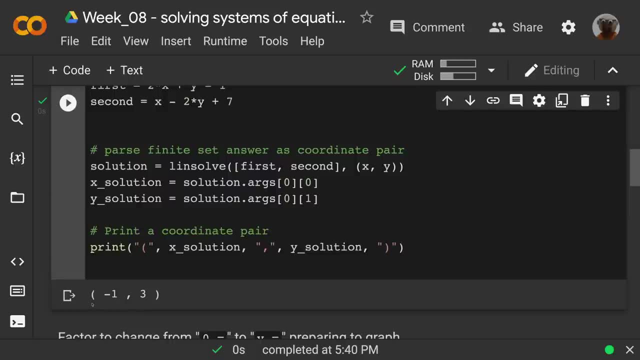 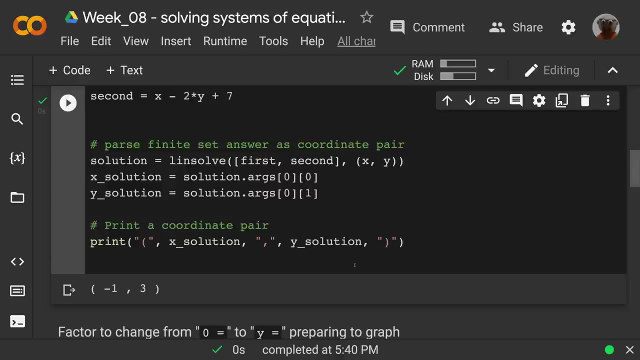 comma y solution, the closing parentheses. and then when i run this, there we go. it will print, you know, negative one, three in parentheses, and i can do other things with that now, um, there we go. so what if i also want to see the graph? now this gets tricky, because we can't. 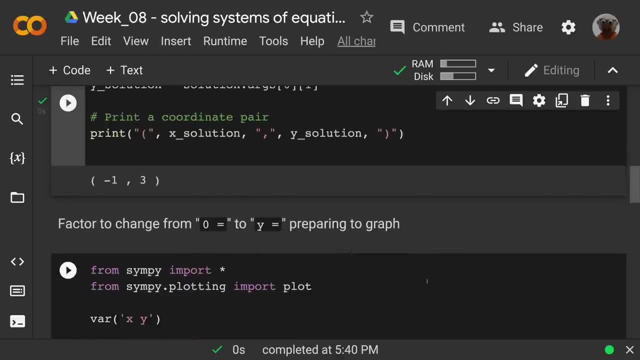 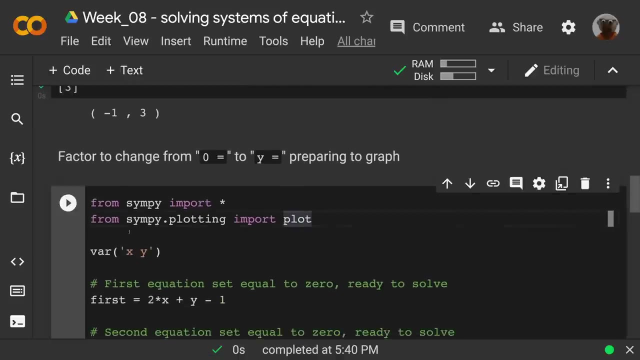 graph the same way that we would otherwise, because going through loops doesn't really work with simpi. going through numpy doesn't really work with simpi, but simpi has its own plot that we can use. so there we go. it doesn't work with the others, but 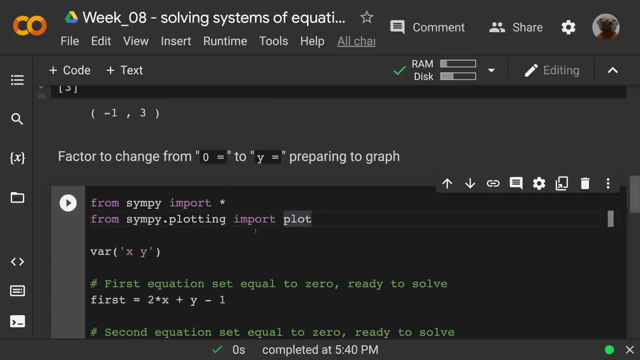 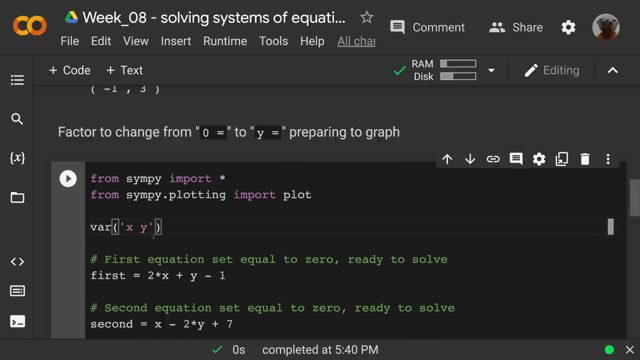 it has its own. so from simpi dot plotting i'm going to import plot, and so this is the simpi plot and, slightly different way, i declare these variables here: var x, y, here. then this one is similar to what we were doing here, so i'm going to import this one and i'm going to import this one. 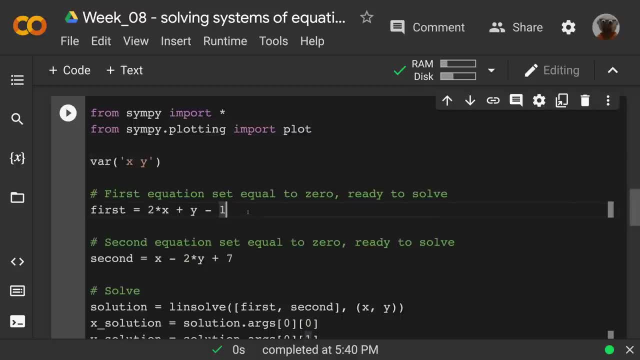 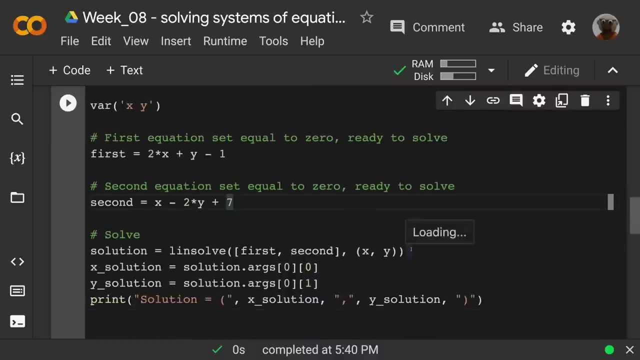 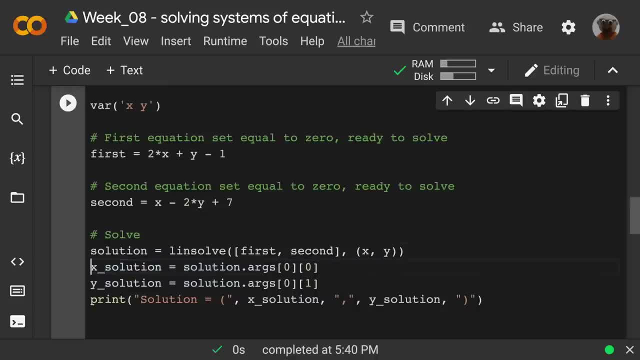 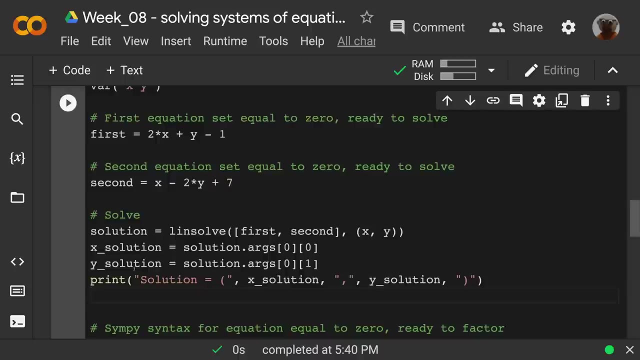 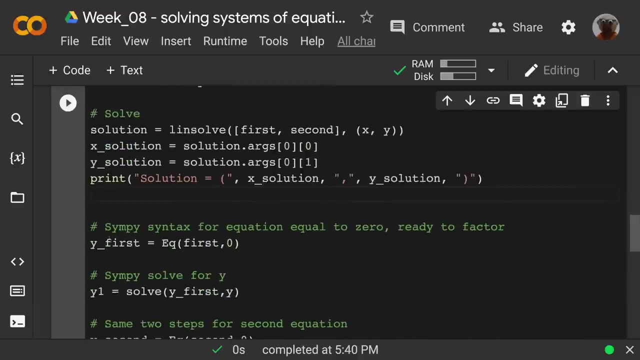 you know, get the solution, um, get the solution, get the x solution, the y solution and print. so this is what i just. this is all the same, what we just did before, but what the other things that we can do is now that i have these, and i know that these are equations set equal to zero. now, simpi syntax. 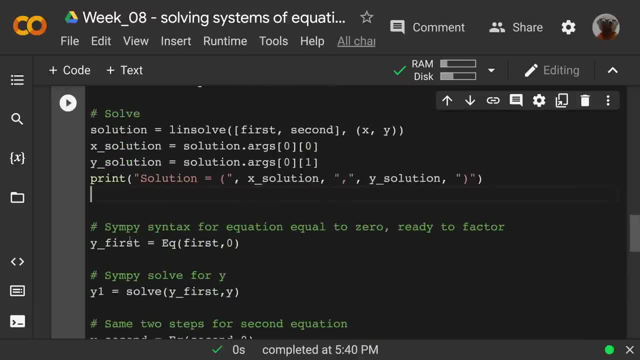 for something set equal to zero. if i want to get it ready to factor so my y value for the first equation, i call it y first. so in simpi we're going to define this as a equation first and then comma. zero means that's that first equation and i'm just spelling it out that it was set equal to. 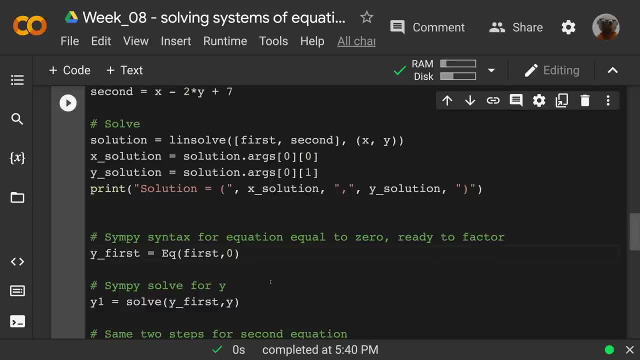 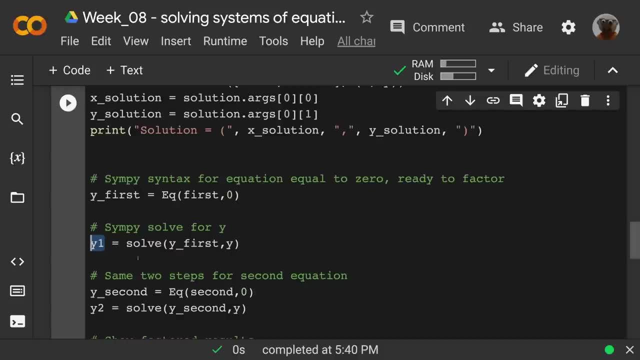 zero. we kind of need that. so now y first, is that set equal to zero, and then y1. i'm going to make this variable y1, which solves that first equation. you see y, first comma y. so i'm going to take that here, spell it out that it's set equal to zero and then do my algebra factoring. i'm going to solve for. 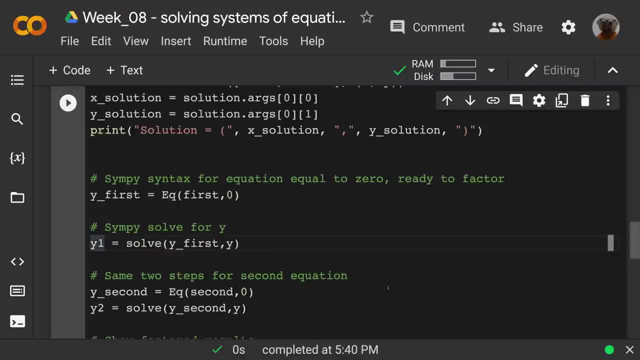 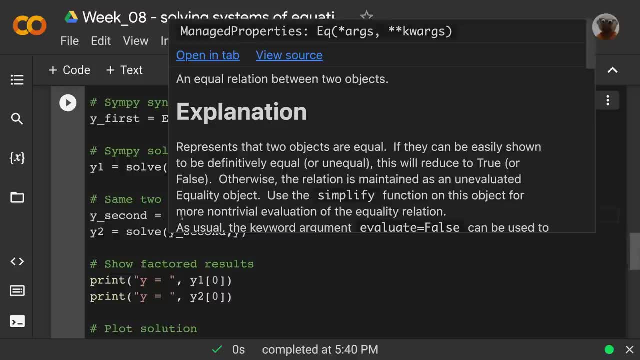 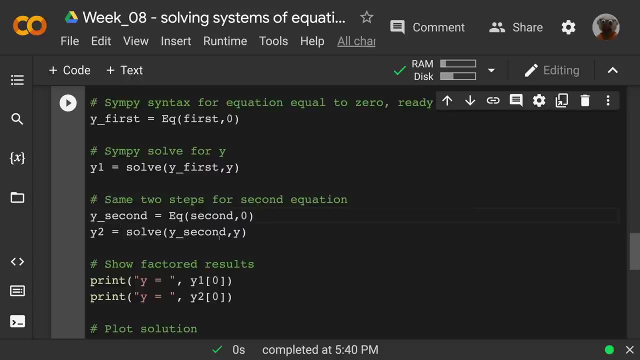 y and then store it as this variable: y1. i'm going to do the same thing for the second equation, so set it as an equation second. the second equation is comma zero, y second, and then i'm going to solve it: y. second comma y. i'm going to solve it for y. so now that i have y1 and y2, i can print them. 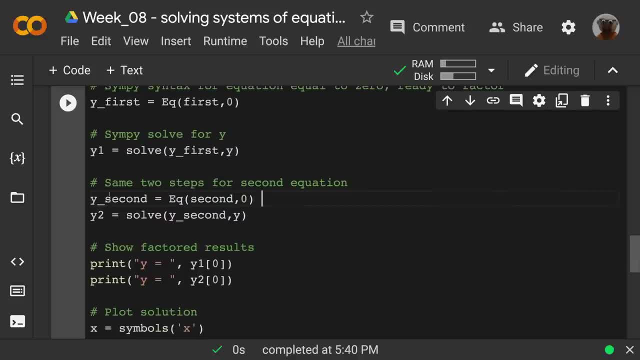 because that might be interesting. so it's just going to give me these. so i have y equals, that i will display exactly comma. and then here's the variable y1- zero and y2 zero again because you know the index of the array. so we have these that i can show factor. but we were talking about graphing this, so let's do that next. but now 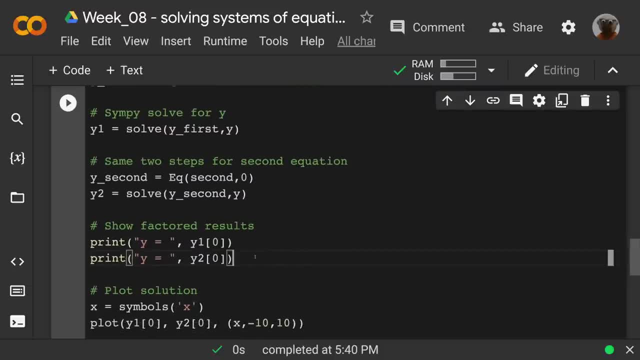 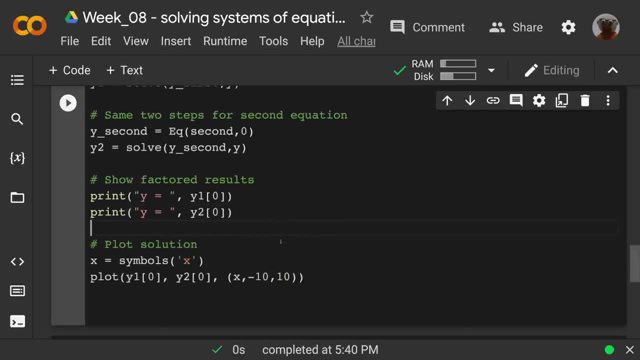 i have. i will display the solution. i will display these, you know, y equals equations, and now when i plot the solution, i didn't just factor it to see that as y equals, though that is really nice, i actually usually like that. but to plot the solution here, see. now i'm going to just 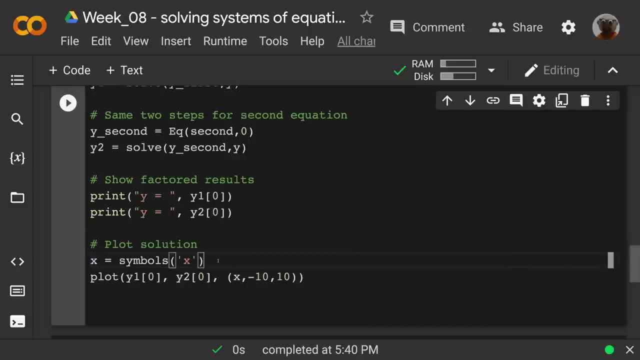 reference x as a symbol. and then take a look at this. i'm going to plot, but notice nothing. dot plot. this is just plot within simpi plot. and what am i plotting? this y value y1 zero and this one y2 zero. so there we go. so when we factored it into, y equals that. 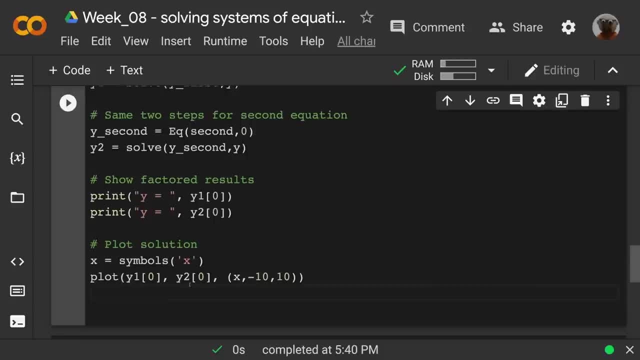 helped us not just display the solution, but put this into here that this is what i'm plotting, these two y equals equations and then the x value. notice also a little bit different the way we display x, comma, negative 10 to 10. i could, you know, make these other variables, but that's going to work out just fine for us. 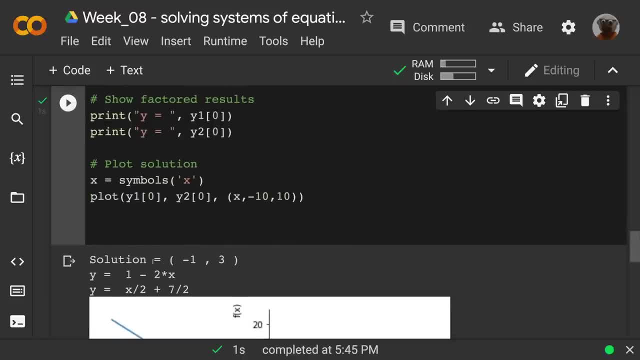 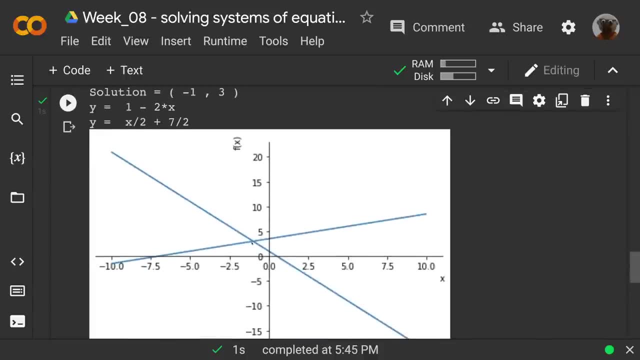 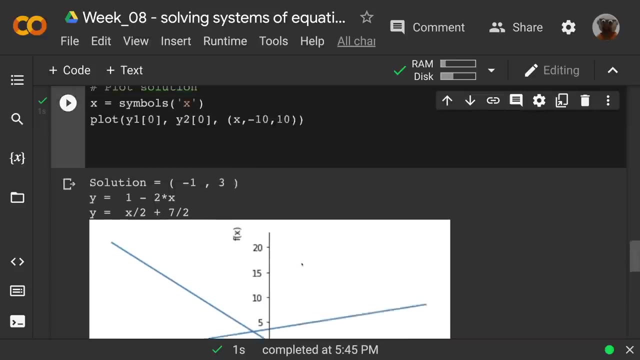 so then when we run this, i see the solution, i have it as y equals, i have that one as y equals, and then i see the graph and we see where the solution is negative: one, three. there we go, so we can do this, for you know any other ones here. 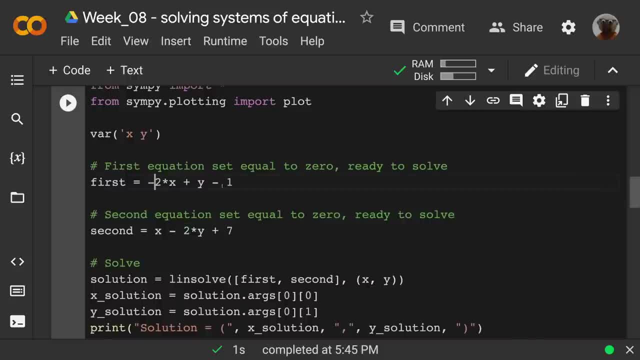 there we go. let's just change it up. maybe make it negative two x, you know, minus two, and maybe this one make this like two times x and i don't know, like plus eight. change it up a little bit, and so we have our first ones and we'll solve it. 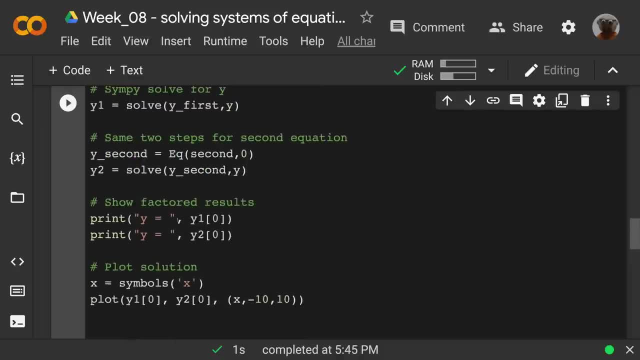 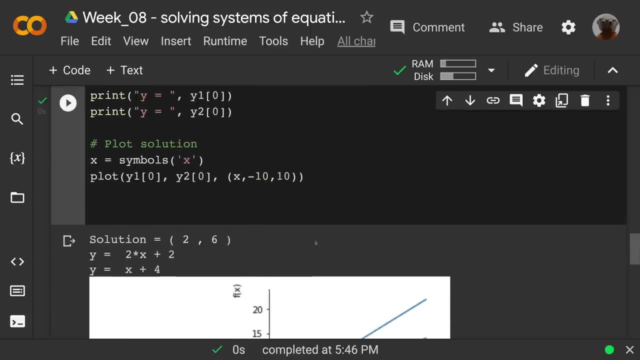 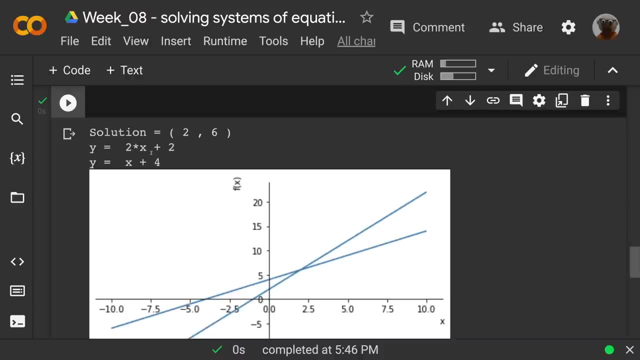 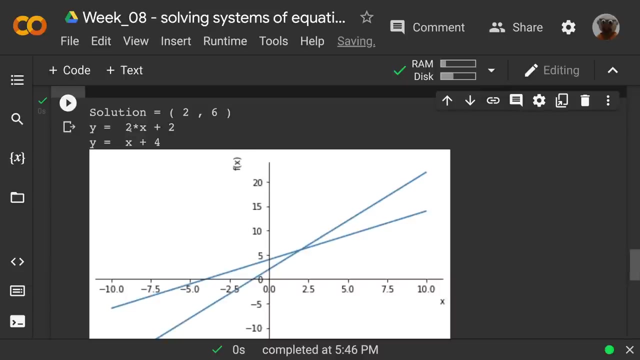 print out the solution factor. it show the y equals equations and then graph it. and now we have this new one. two six is the solution. here are my two equations: y equals two times x plus two and y equals x plus four. so we see these two and how do we know which one? 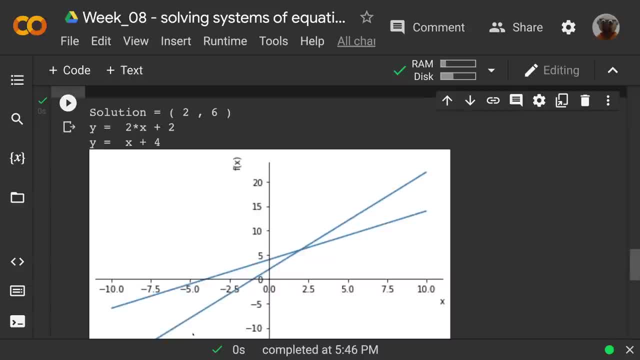 the two times. x has a steeper slope, so that's got to be this one. that's the bottom line. and then x plus four, the slope's only one, so that's got to be this top line. and we see that they intersect here at two, six. 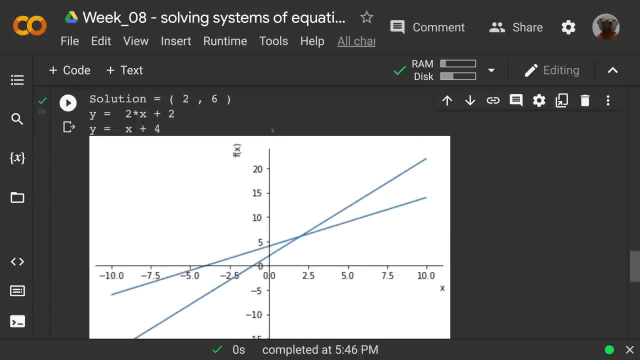 all right. so we see how we can solve and we can solve and graph. there we go, and this works for linear equations, for uh, equations beyond linear. we'll cross that bridge when we get to it, which is going to be in the upcoming sections. now that we've worked through the array of equations, we're now working on some of the Fritsch equations. 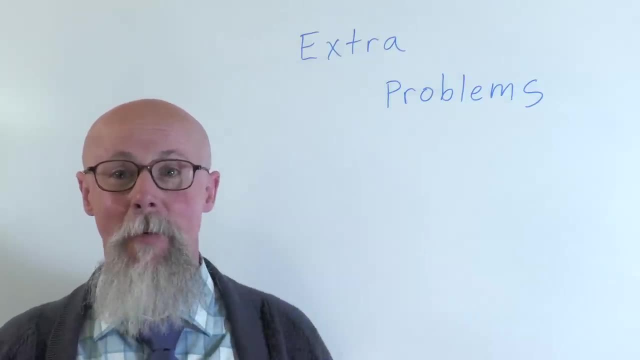 through the core skills in this unit. Let's look through some extra problems, and I'm gonna work through extra problems using the Colab notebook So you can see how you can apply these resources that you're building and use these to solve problems that might come up in a textbook or in day-to-day life. 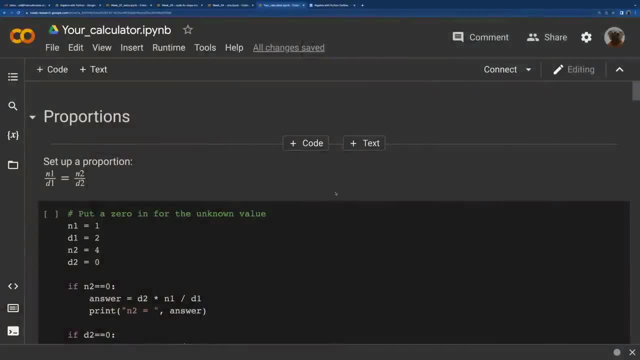 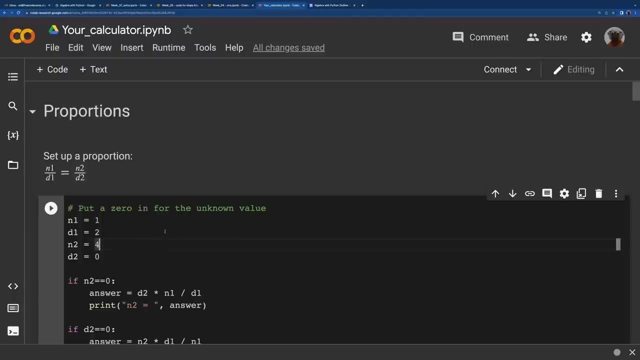 So we're gonna go through some more extra problems here. So here again is where we're gonna put together all the newer functions you've been learning into your calculator so that you'll have these as a reference And remember we already have, or you should already have, the proportions set up. 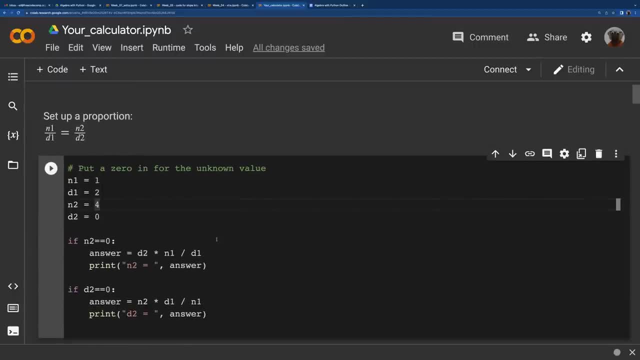 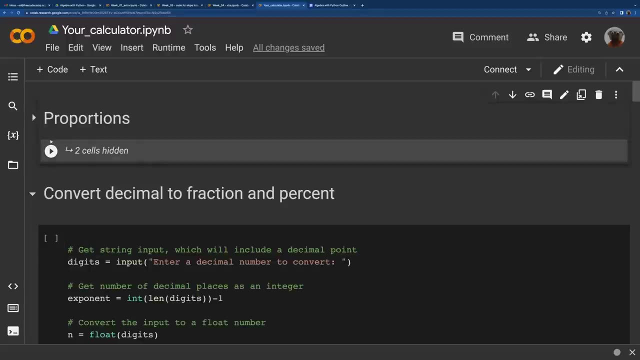 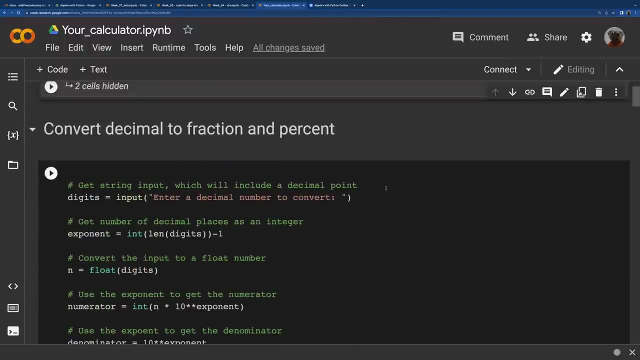 So the text to show the setup and then the code to enter it in and solve your proportion. And remember, we made this a heading so we can minimize that. There we go, And we already did this, converting decimals to fractions and percent. So again all the code there. 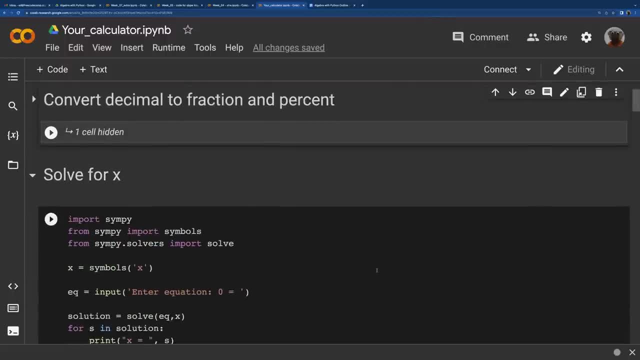 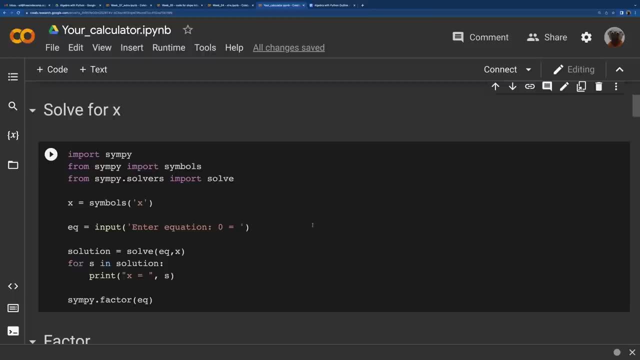 and that's also a section heading, And then we can solve for X. So each week you're learning and we're building, and then we're gonna take like the final product, all of it put together. So here's one, If you just have an equation that you wanna solve for X. 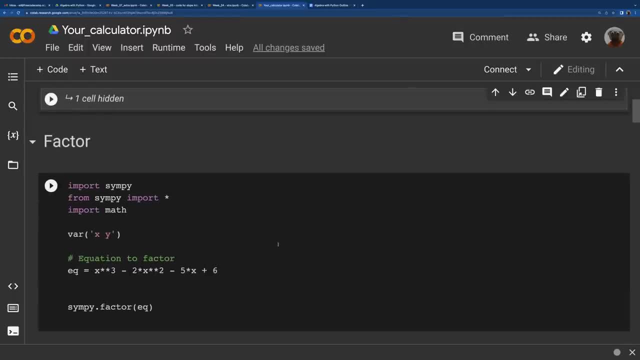 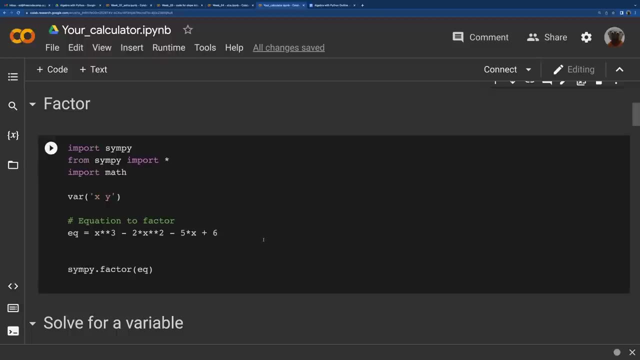 pretty straightforward. we'll have that there And factoring, So we can solve, or we could factor, Factor out a common term or something like that. We have that And each of these. you don't need to use our interface because you just have this: the solving. solving for X. 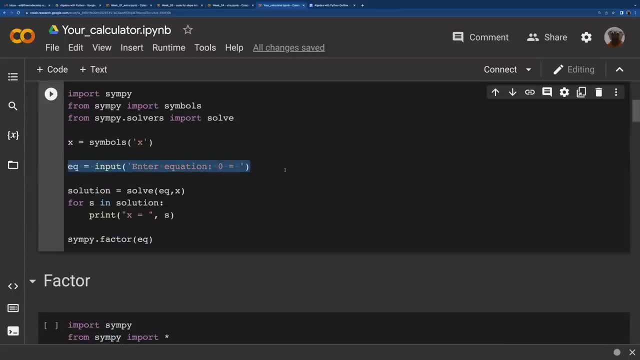 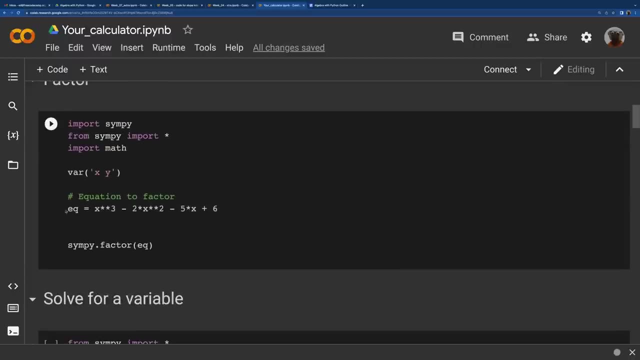 We did put a user interface in there. It's gonna prompt for the input And then you see that the equation set equal to zero, Whereas the factoring one. it's just this equation that you know there to put it there, and then sympyfactor. 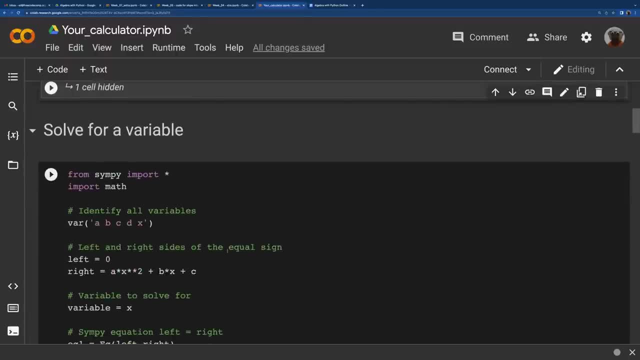 Okay, so that's also a section heading. Then recently we were doing things like solving for a variable, So not just set, solve for X, but even if it's not a definite number, to actually rewrite it. you know, like Y equals A over B, or something like that. 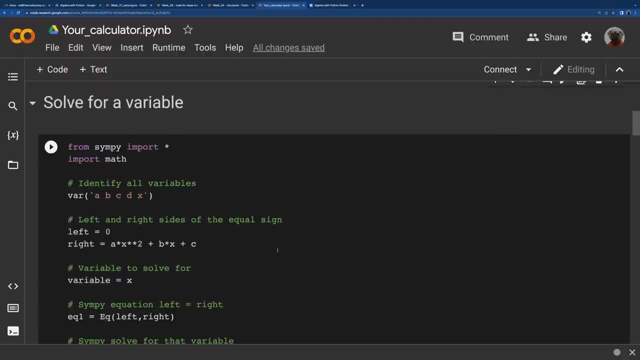 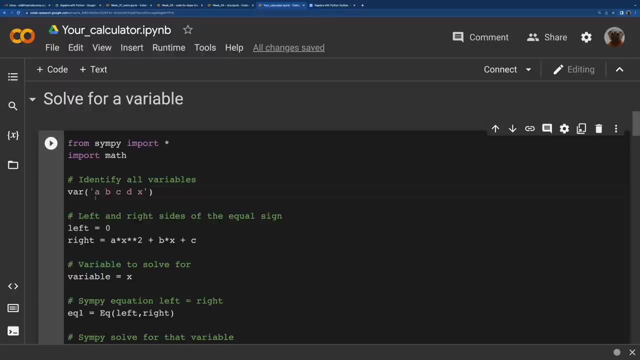 where you don't even have numbers. this will do that for you, And we defined a lot of our basic variables that we might use. It's not gonna be an error to put them in there and not use them, But you could always. 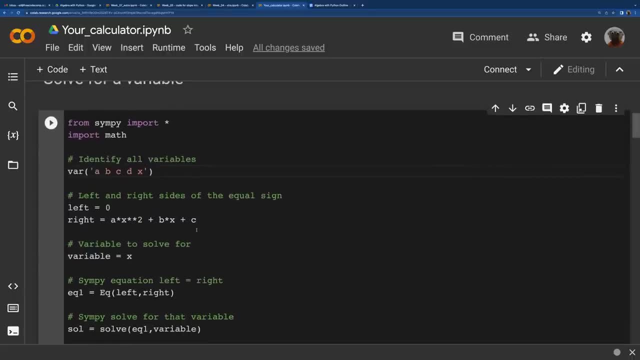 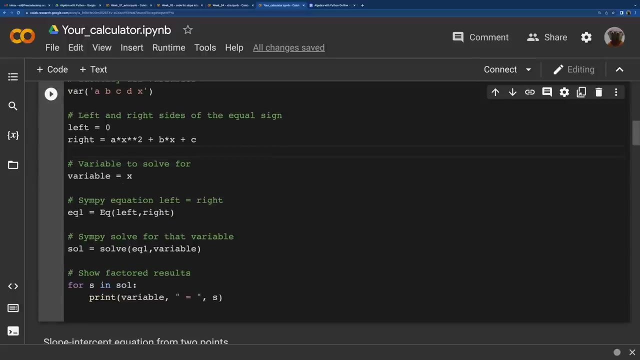 if you change what variables you use, you could always edit that part And then, whatever it is, whether it be involving numbers or a bunch of letters and variables, you know left and right side of the equal sign, And then we have this: 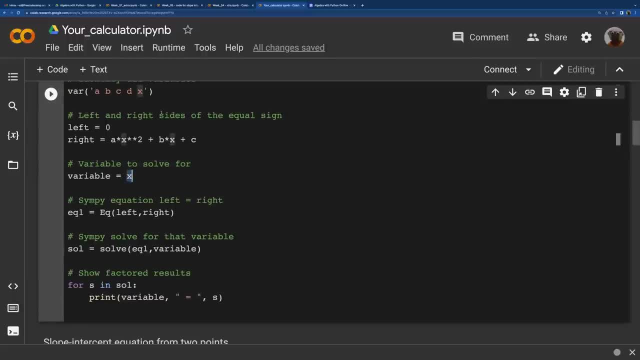 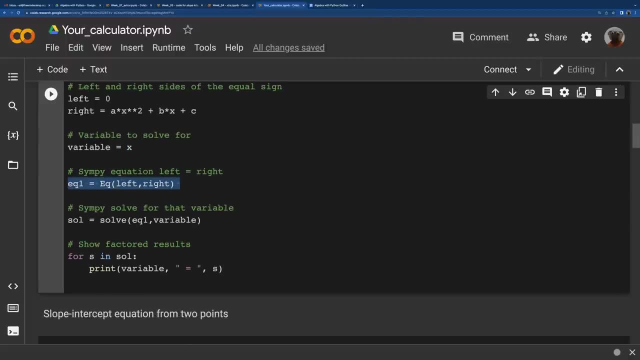 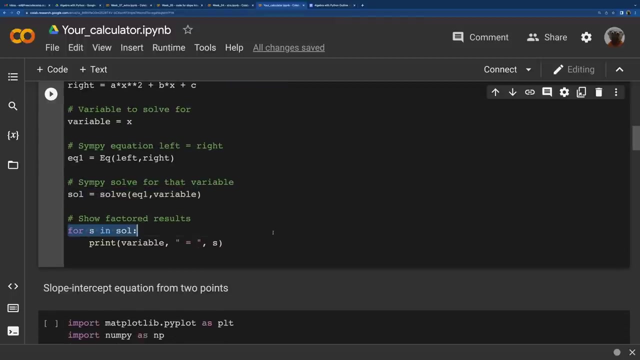 then we're just gonna define the variable So that way you can pick what variable you wanna solve for. set it as an equation- Remember we did this- and then we're gonna solve, and this loop runs through all possibilities for S in solve for solution. 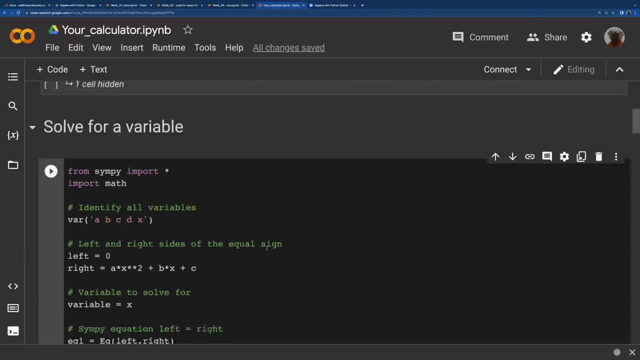 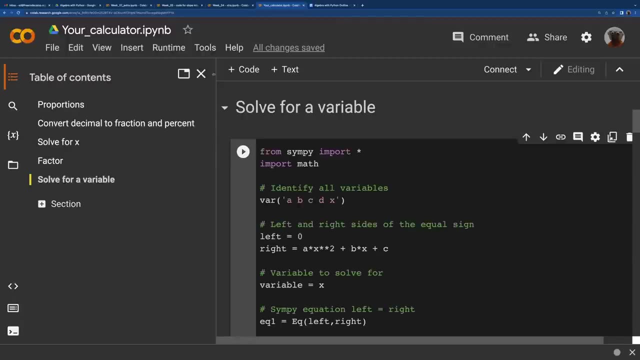 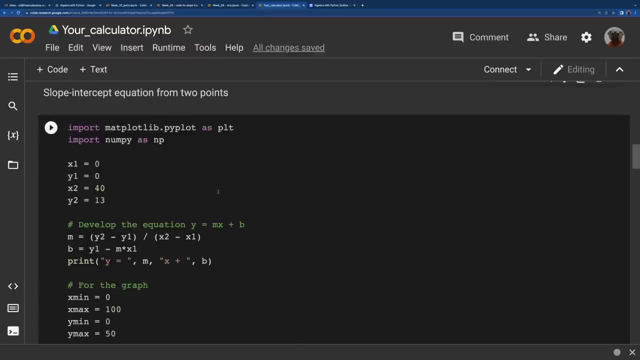 So we have that, that we can solve for a variable. Again, it's already heading and we have that, therefore, in the table of contents. So we're gonna add the other things we've been doing: Slope intercept from two points, because this in itself is a very common thing to need to do. 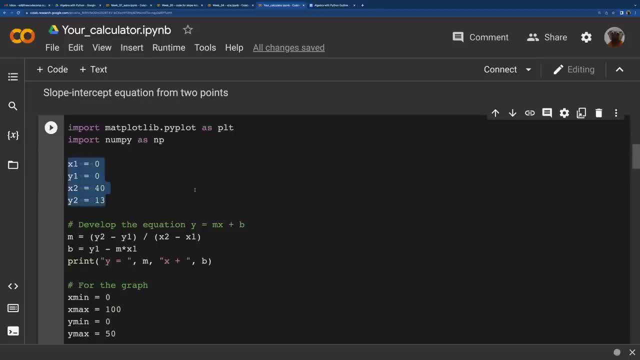 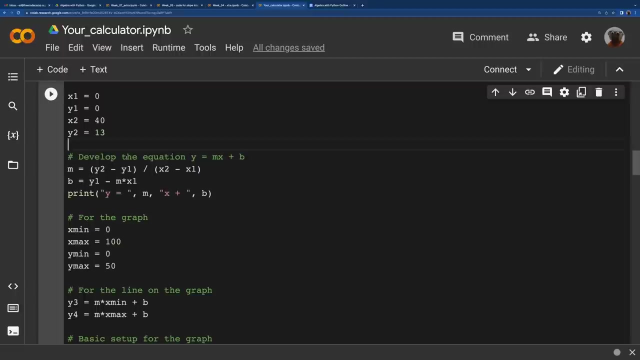 So we're gonna define the two points. There we go: X, you know X and Y, And then, using just our slope formula, solve for B, we're gonna get M and B And having those two, we're gonna print out the equation. 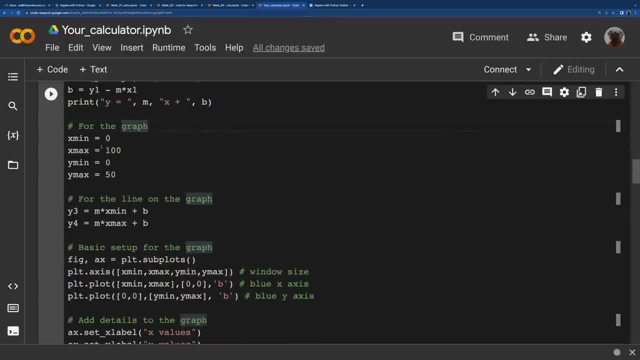 And then we're gonna use that for the graph And you can keep this at these numbers if you want. You know, you could always change this X min negative 10.. And we could leave the others as is, but you could always change them to 10 in every direction. 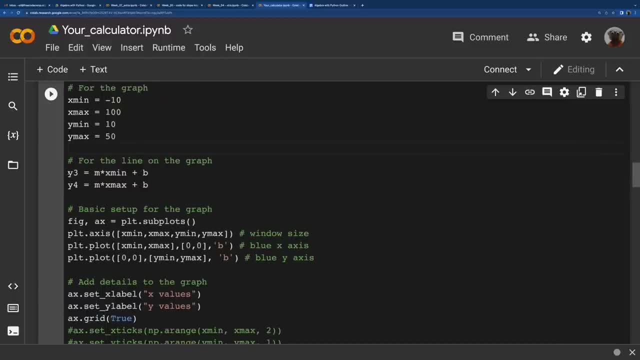 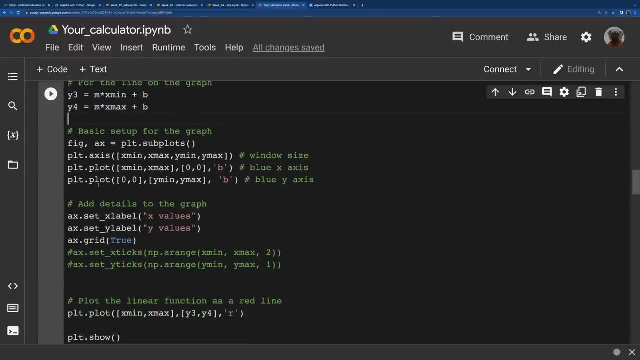 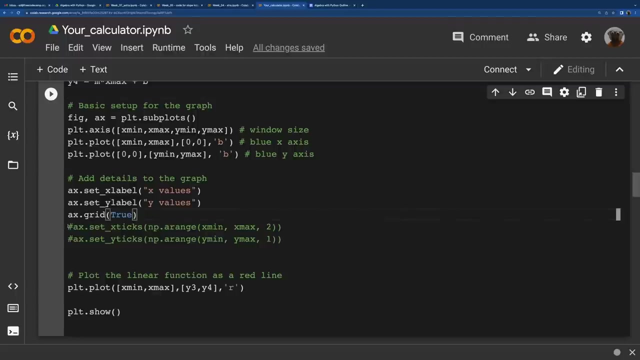 if you wanted to And having those, we have these. you know, for the graph And the setup the details could always add other details or change these And you see, for things that we might use. we might wanna see the tick marks. 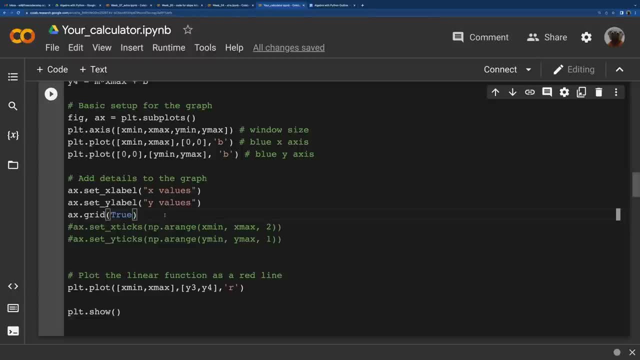 So we have them there so you don't have to really think about. you know the exact syntax. Hopefully, the more you do this, you remember it. But it's just there and it's commented out, So you can use it if you want. 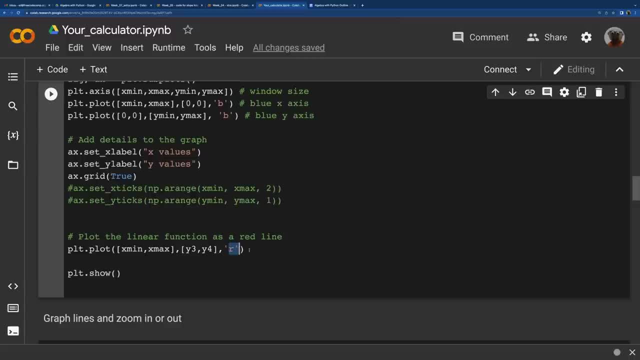 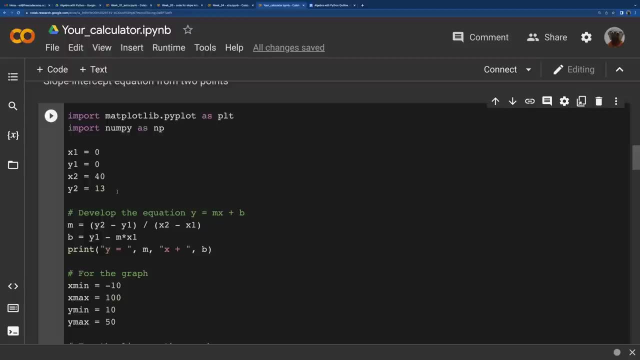 And then that way here we just plot the function as a red line. So even if you end up changing some of these, you have a lot of things that are there by default that if you really entered in two points, you could solve whatever you wanted to solve and graph it. 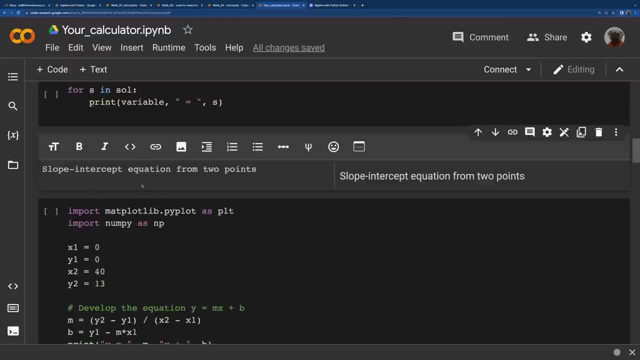 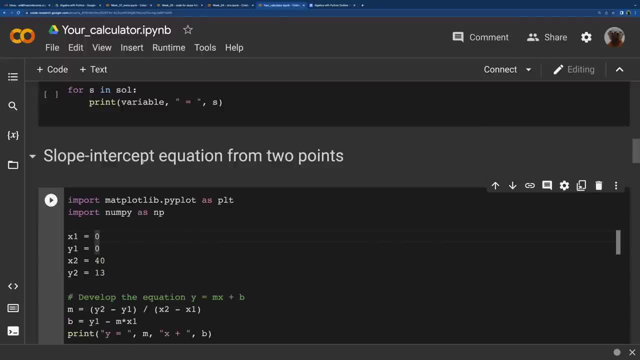 So we have that here. Let's make that a section heading. then We can double click And remember it's this hashtag, because it's in the text, not in the code. Now that became a section heading and shows up in the table of contents. 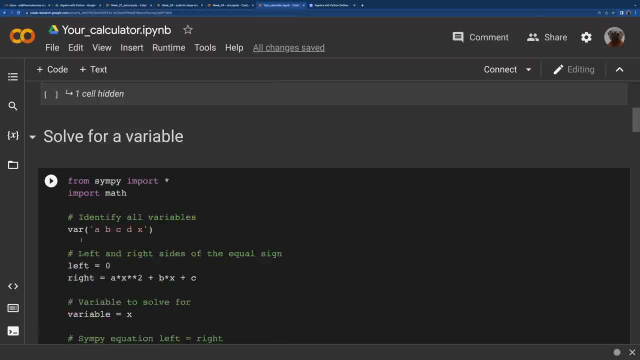 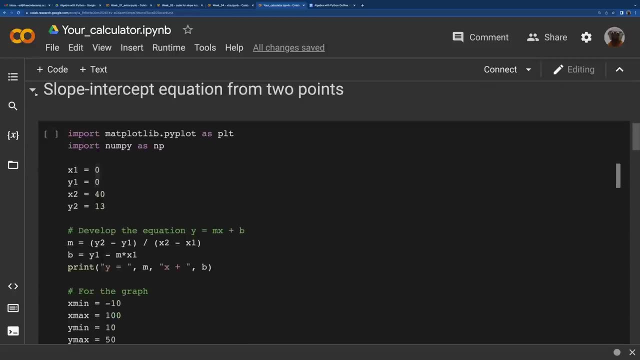 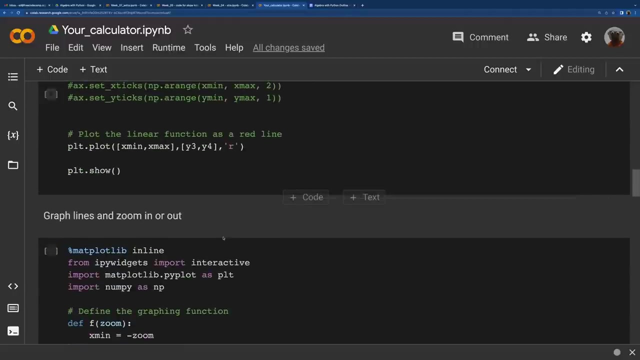 So we have that. Now the section heading goes all the way down to the next heading or the bottom. So that one we can minimize now This one. if we minimize it, that's all the rest of the document here. So besides that I might just want to graph something. 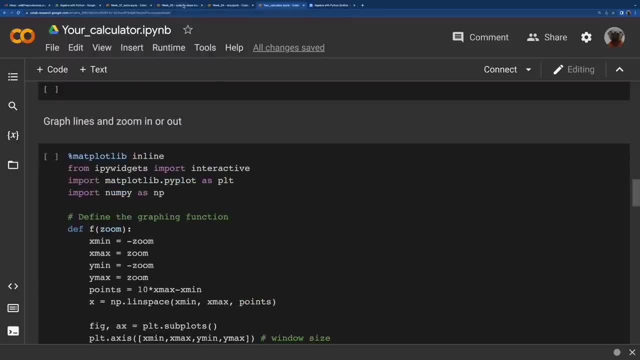 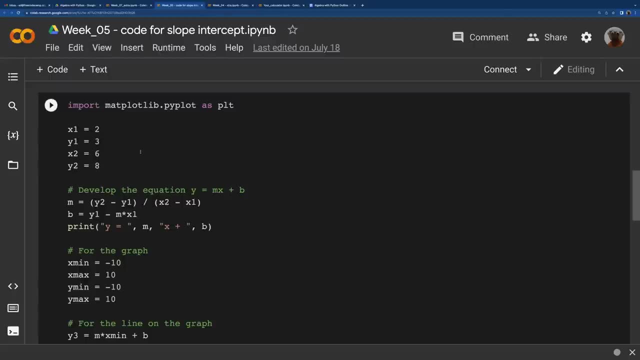 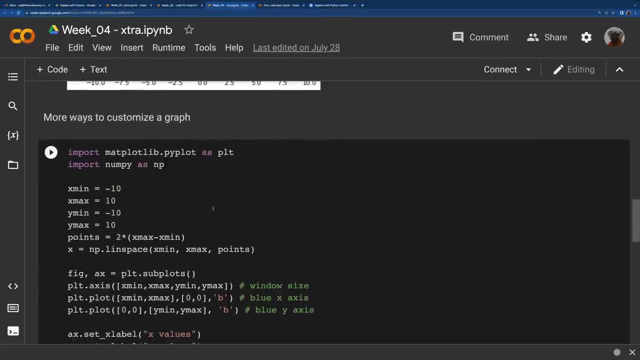 And remember in you know we use this, the other code as you're building it. remember the slope intercept stuff came from week five and then other ways to customize the graph came from some of the extra things we were doing in week four. 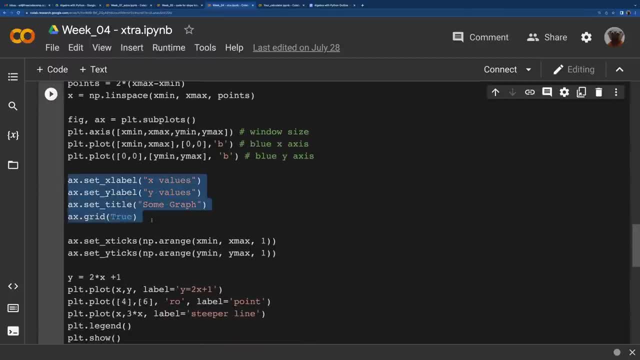 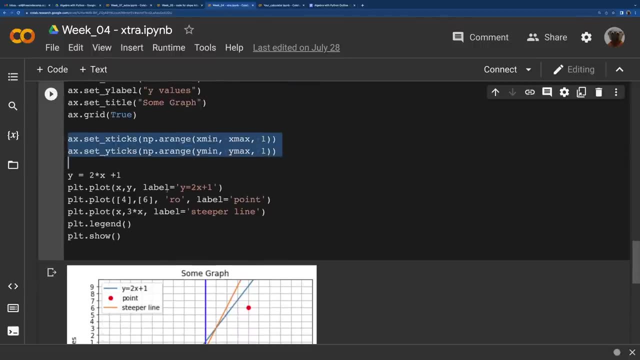 where we have, you know again, all the different things we want to do with the graph, the labels, As well as setting the tick marks And this one, you know, we even customized the labels down here, you know, and added a. 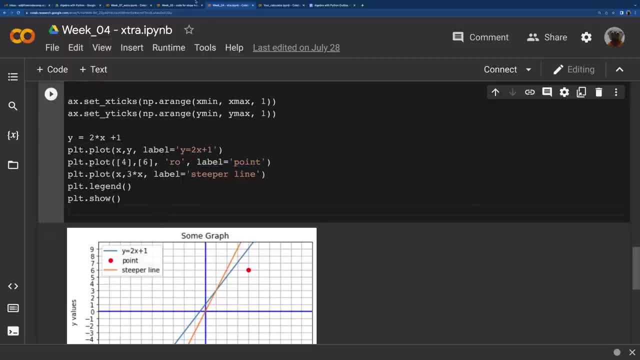 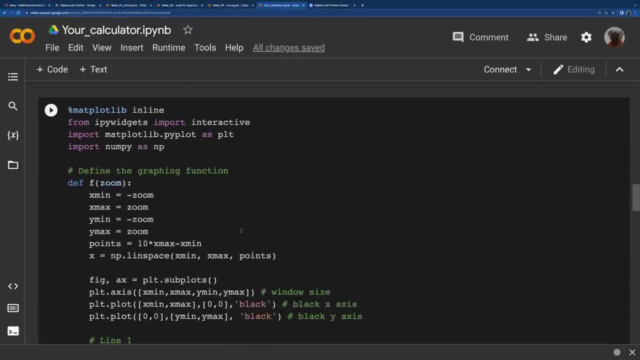 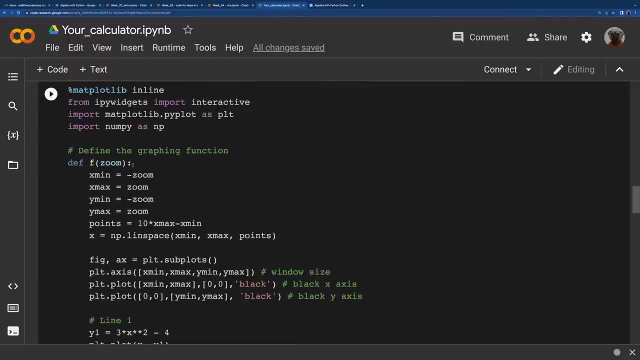 remember, we customized it and added this whole legend here, But in copying this for yours, we're going to put all these, as well as the zoom that we were doing, all in one thing, So the function then does all the graphing. 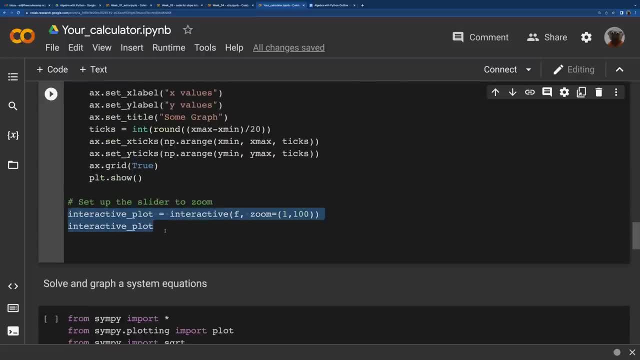 And I'm going to skip down here for a second- The slider. remember that interactive plot. we're going to run this, function F, and the only slider we're going to have is to zoom, And that's going to be our multiplier from one to. 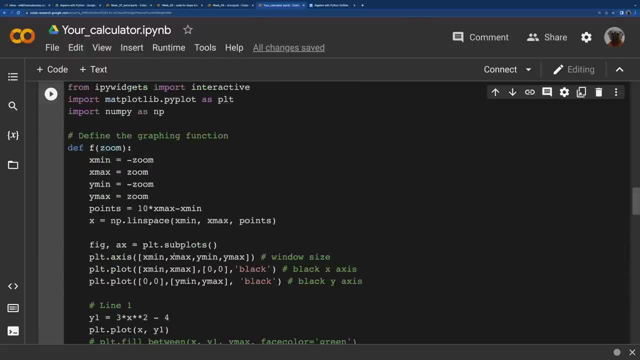 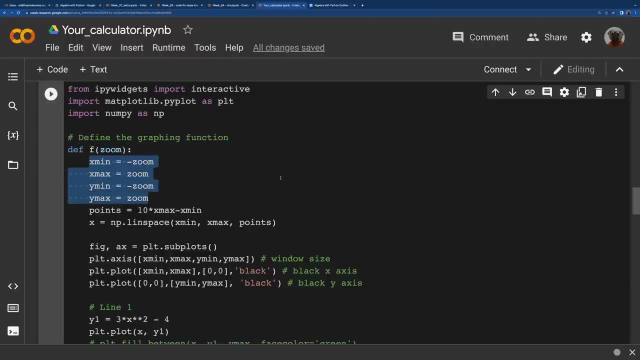 I just picked a hundred, That's good, And then taking that, so whatever that multiplier is, that will define what we have for our X min and X max And then, once you have those, we can define the points for our nplenspace to graph. 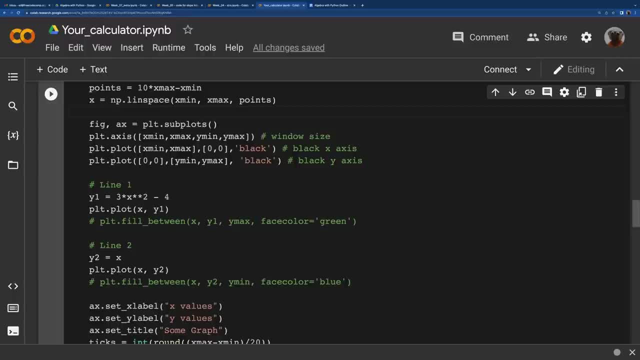 And there we go. And I just put this. you could do the same, just two lines, as by default. you know, maybe you want to have two lines and then you, you know, you want to see where they intersect. So this graph's two different lines. 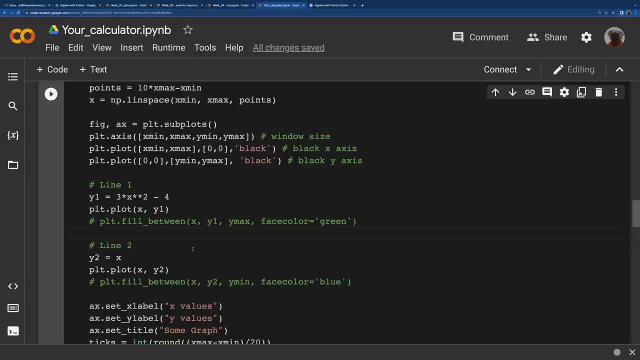 and notice, does not have to be a linear equation. So, as long as you're using Python syntax, whatever line you want to graph, And we- I commented this out, but again you could have it if you want to fill between shade above or below. 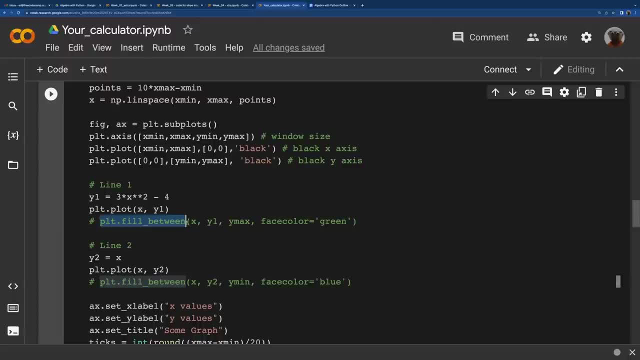 And I just happened to have this one fill between same X values, So the Y value goes from Y1 up to Y max, And so that would shade above and it would make a green. And the next one Fill between same X values from Y2 down to Y min. 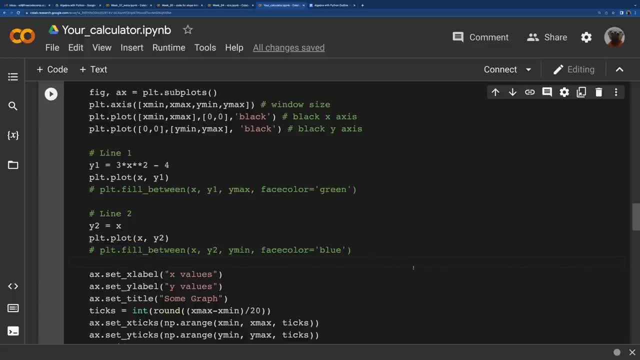 and then you could just put those up for X value, I guess. So now that we have the Y value, it blue, so that would shade below. so again, you could have these here in case you need them. we're making these default uh notebooks that you can use and you say: oh, okay, i do want to shade above. 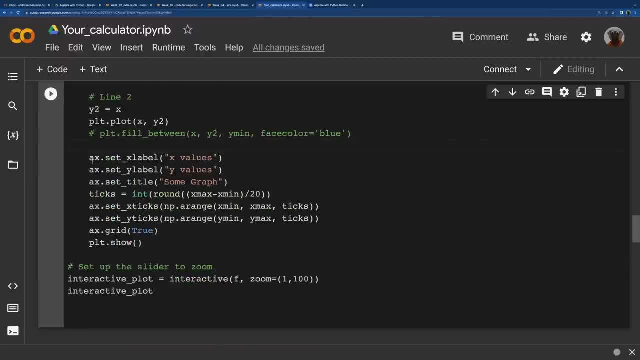 or below, uncomment it. and then we have the labels, general labels you can change. now for this one, i kept this, the tick marks in there and the grid, and notice, because a lot of this is based on the zoom. so then, how many ticks do i want? and what i did is i got the difference? 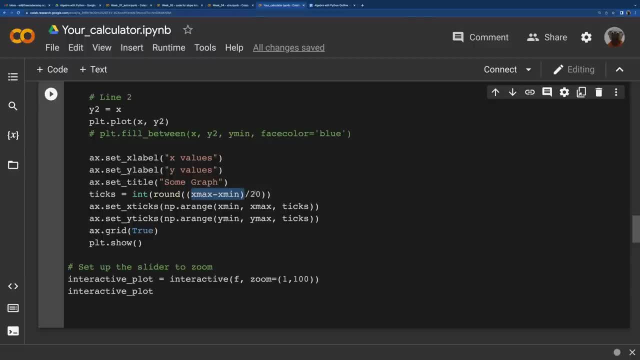 the how you know, from x max to x min divided by 20.. i tinkered with this and that seemed to be a good number to display nicely. so we're going to get that divided by 20 and then round it and then cast it as an integer. so the number of ticks has to be an integer. 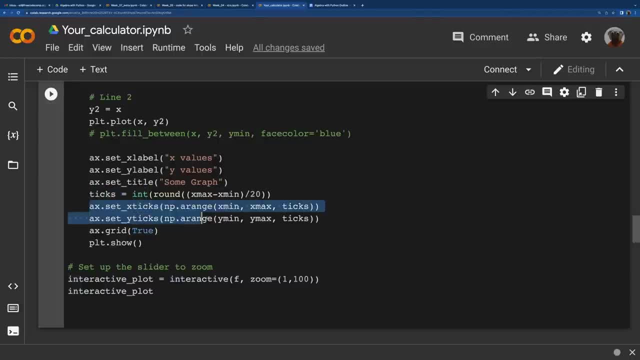 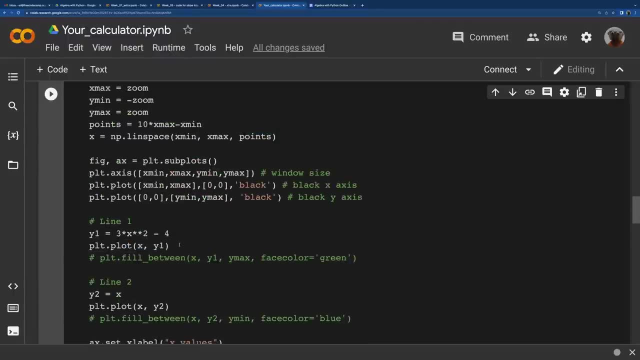 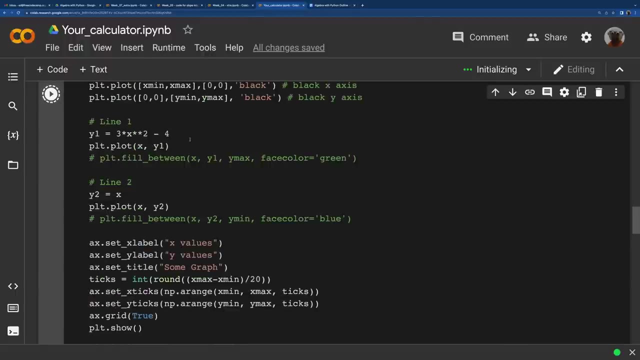 so then that way, no matter what the zoom is, you'll see that we can adjust the tick marks and show the grid. so this will give us a few things that we can graph. you know this default. and then let's see. given these equations that we have in here a lot of times i like to keep an equation in there rather than just like make. 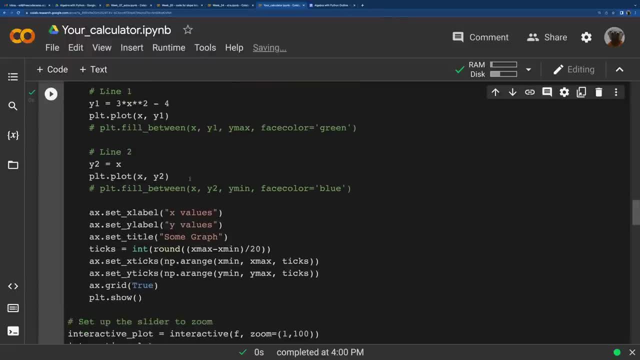 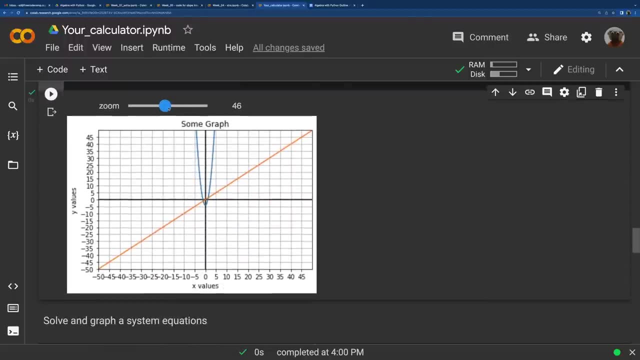 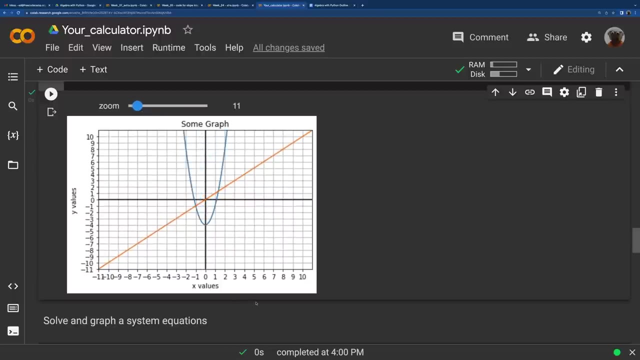 that line blank. so if you run the code, it works and you see something. so here we have this graph and we see the default zoom goes right to the middle. but i can move this back down and you see everything adjusts. the tick marks adjust, the graph zooms in and then we can see, you know, or we can zoom out. 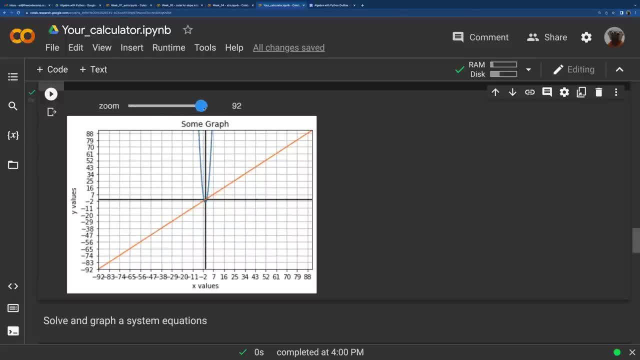 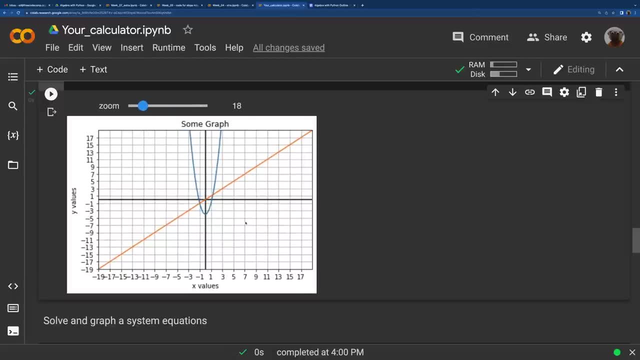 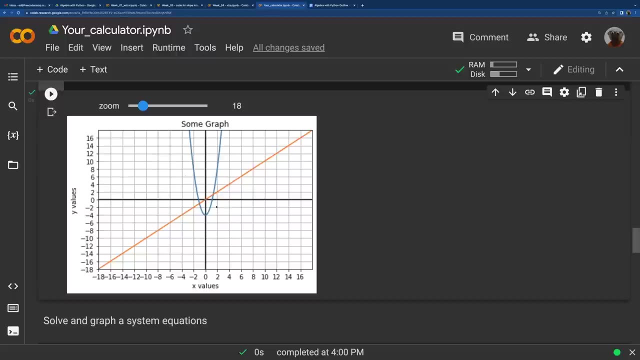 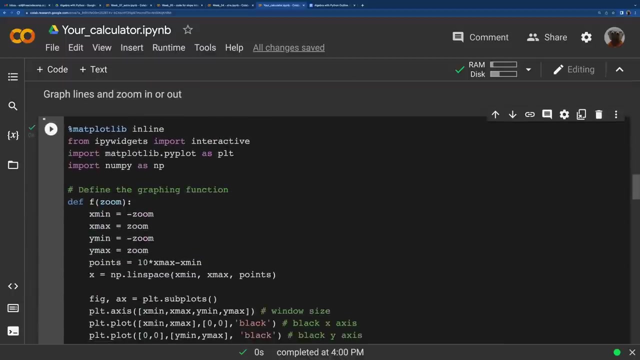 and we see. so, yeah, pretty good. i like kind of for this particular graph, i like it zoomed in and then you can see, you know about where they, where they cross. so sometimes you just might want to graph something and there, there we have that and there we go. we could put more directions and you could have the whole, ever, all the directions. 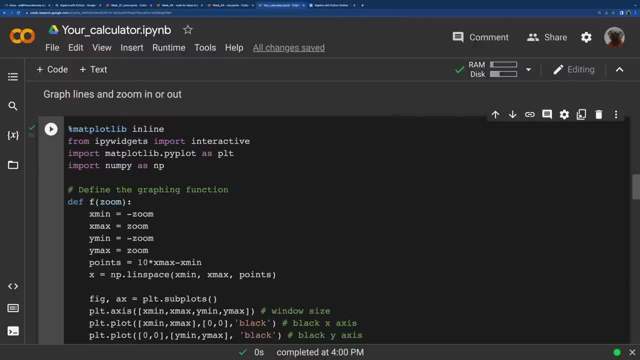 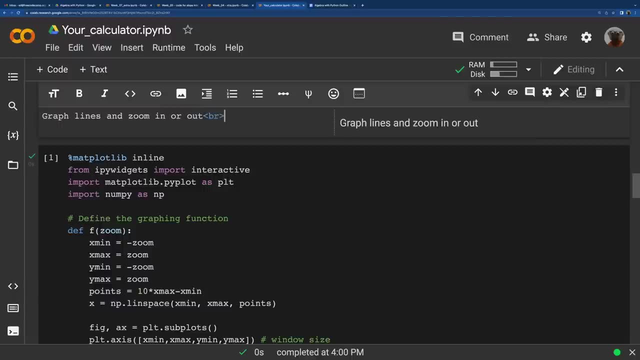 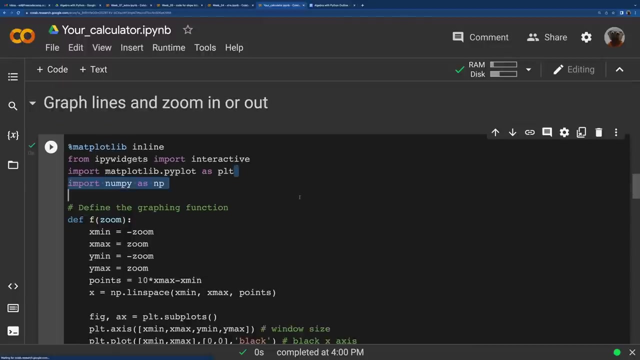 don't have to be, uh, the heading. you could have that and you could put an html break, um, right after that if you wanted to, and then more words underneath. that would not become a part of the heading, but for this we can just put the heading here. there we go. i remember there's really no. 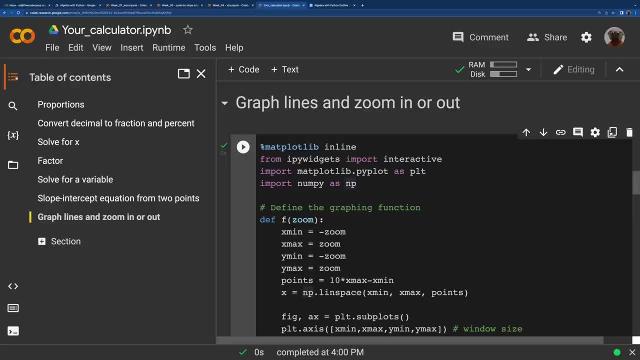 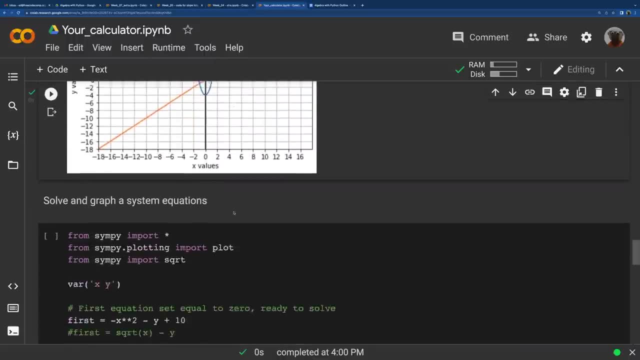 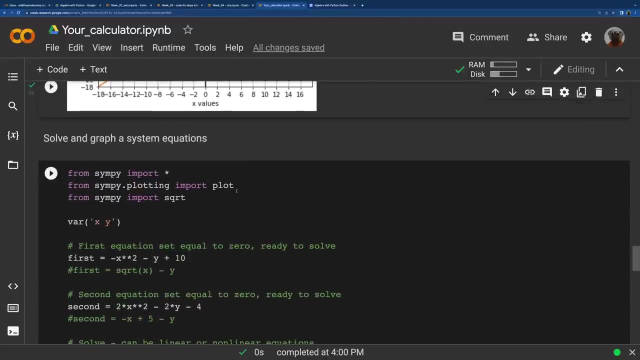 entering would just put it on a little line. you just click somewhere else and now that's also a part of the table of contents. so we have that and then solve and graphic system. and this is nice, it brings it all together, solving it and graphing it. so here you can put in as long as you have python syntax. whatever you have, there is your first. 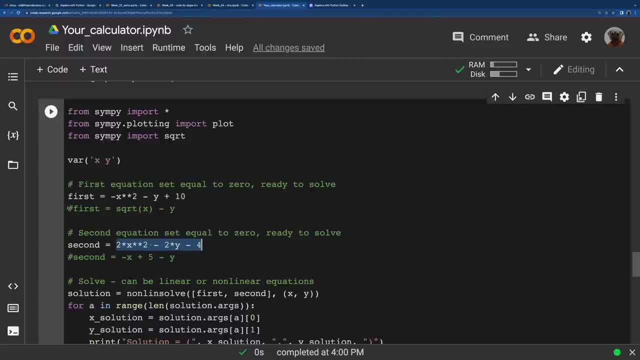 and second equation- and i even have an extra one here just to be able to uncomment, and you can see, this will even work if you have a square root. um, just to have different ones to show you, and we've used the lin solid and we've used this. if you need to, uh, i just i'm gonna tight. 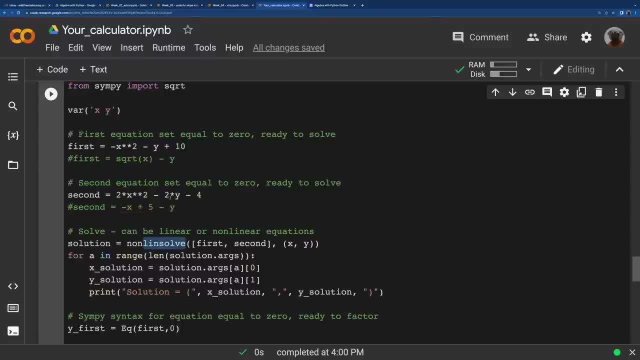 it and then just flicking it up and AMD transmit it straight to this so that we can see: um now, if solve before to solve using SymPy, the Lin solve to solve two equations, And this is actually another one non-Lin solve. I like this one because it can be. I just put the comment in. 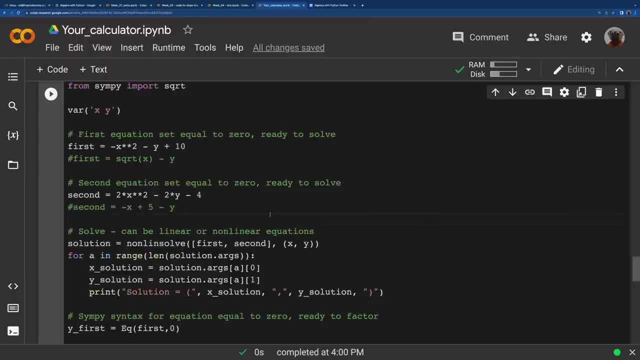 there. it can be linear or non-linear, It works out. So just because you have non-Lin solve does not mean that you have to have. you know something different if one of your functions is linear. But there we go The comments, just so you know. here's where you enter in. 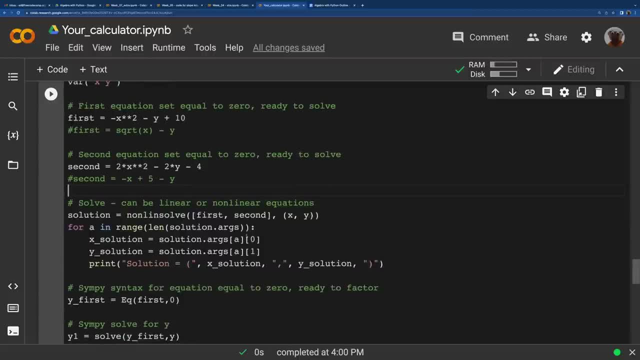 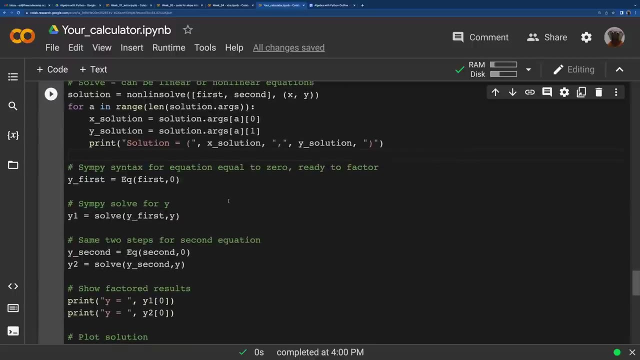 and then you already have the code that you would have copied. This one would have been from eight, yeah, from the recent week to solve and graph. You can just copy these and then tinker with them a little bit, you know, as we went through and built up to these important. 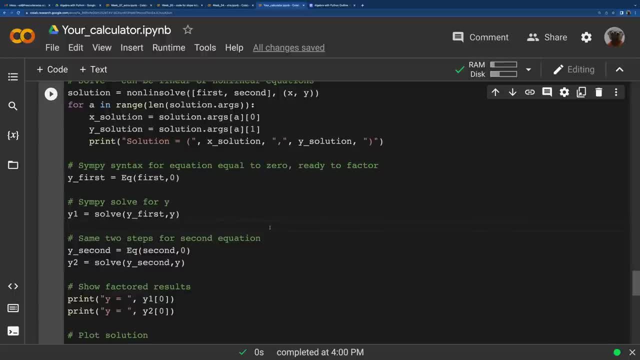 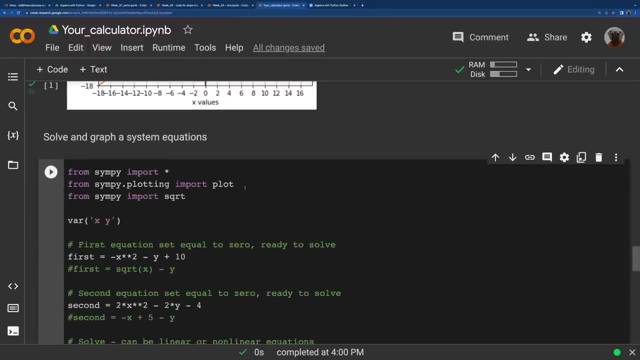 um, uh, blocks of code. you know, take the last one that brings it all together and then put it over here. You know that's what you're doing. You're building your, your library here. So solve and graph the system of equations, and then this will work. 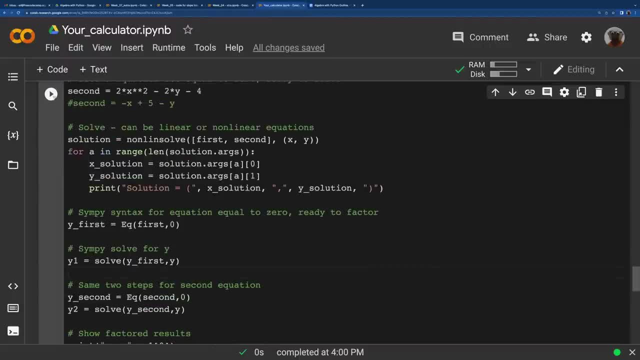 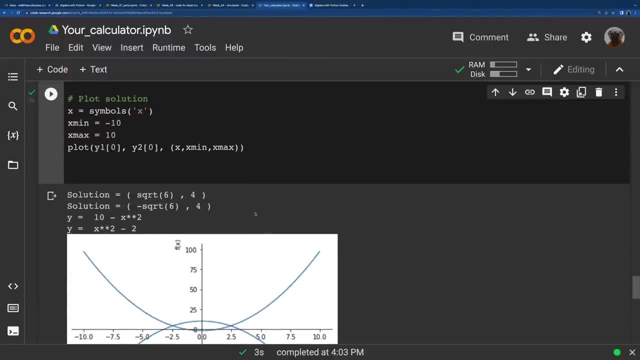 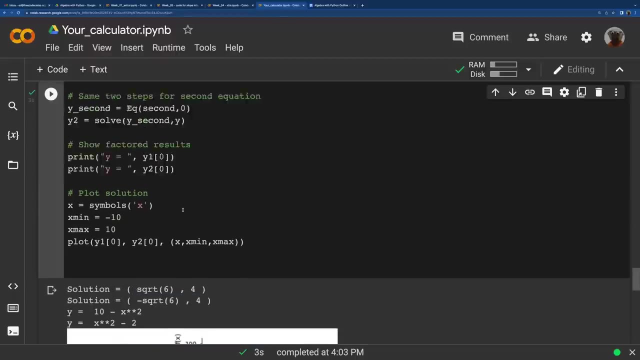 Solve and graph pretty much anything, and I just want to show you some of these. So, even if it's non-linear and you see, it'll give you the solution x, y. this one happens to have two solutions. Um notice, because we had the uh. 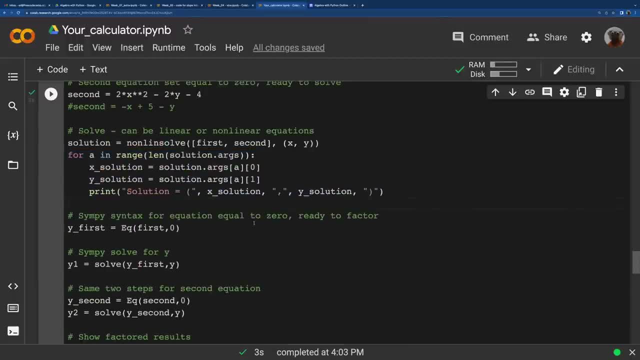 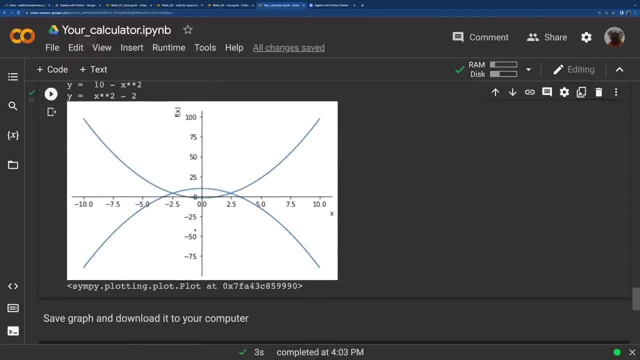 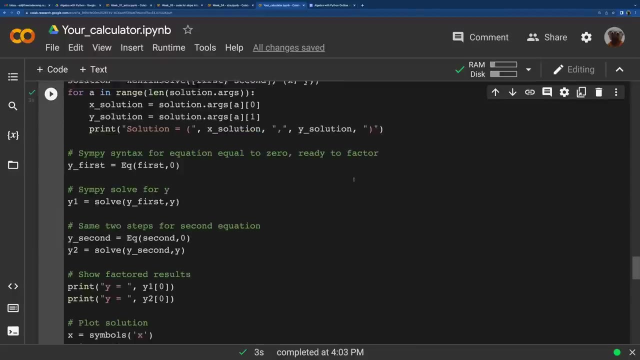 the loop, the for loop, here to account for multiple solutions. So it'll have the two solutions, then also show the two y equals equations and then graph them. So that's pretty complete. That's a good, good one. You want to have this as this type of thing in your toolbox. 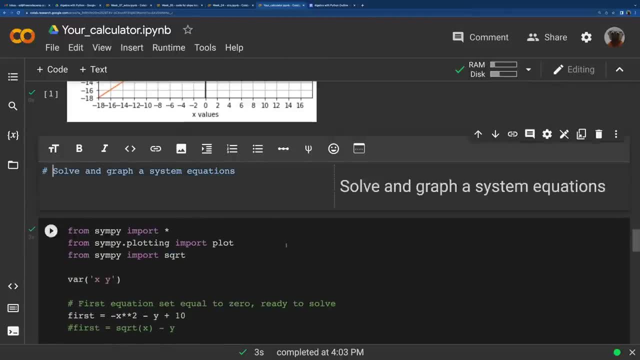 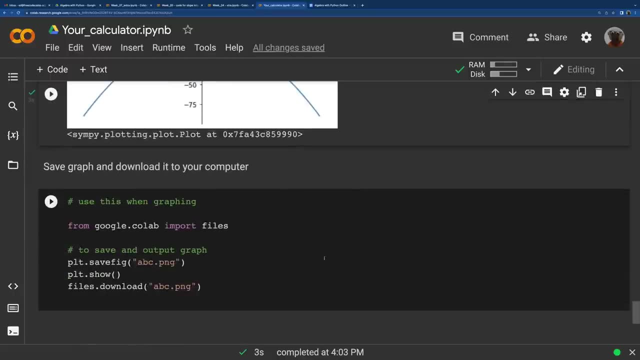 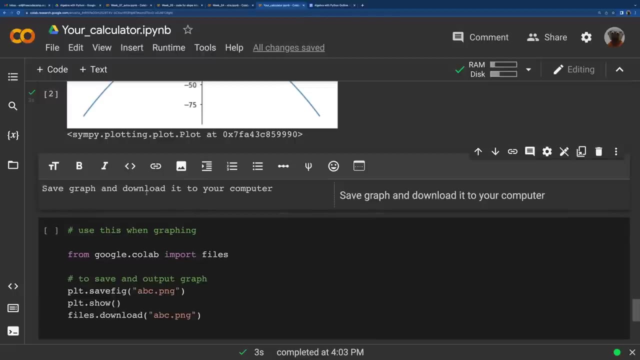 Double click and let's make this one a heading. There we go. So we have that, And I've added one more thing here, Um, and we could still make this a heading. Notice: this code isn't complete, but I put one thing in here that give you a reference point, So you certainly 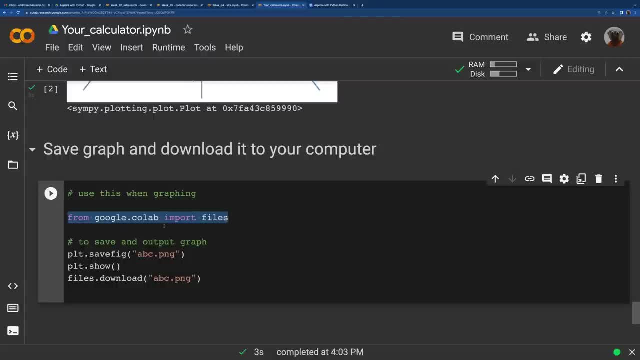 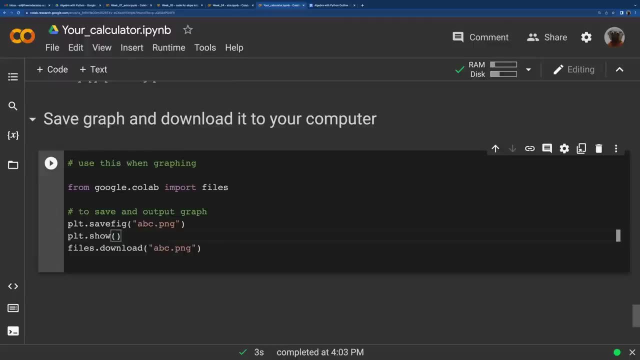 you would recognize that that's import. So that would go first, And then you see, this you would also. it would be something you already graphed, So the PLT would already work. but notice, you have this, that save fig. 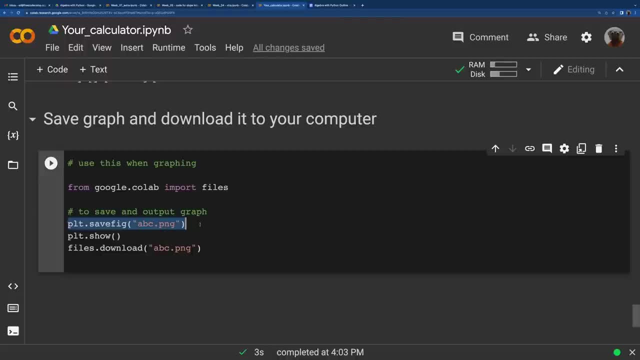 and you're going to give it a name dot PNG. That's a good file type to use. Notice that'll come before the PLT dot show And that actually works If you put it after. I've tried this. if you put this after, it actually will save something, but it'll be a blank graph. 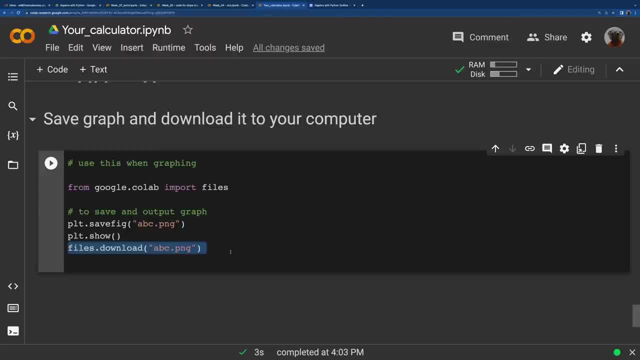 And what's interesting is this download can come after. So that's okay. I mean, you could put it first, that'd be fine too, but it can come after um, because it doesn't interfere with what this shows. And this is a way to download this to your computer or your phone. There we go: Save the. 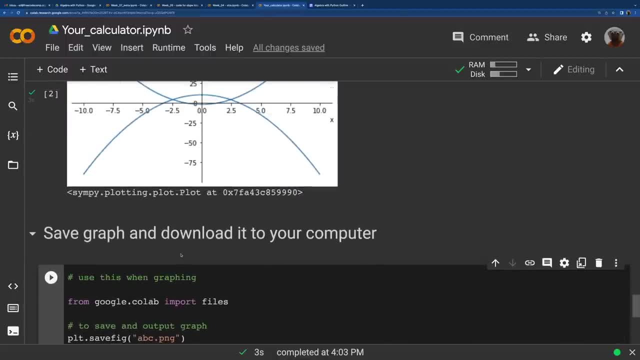 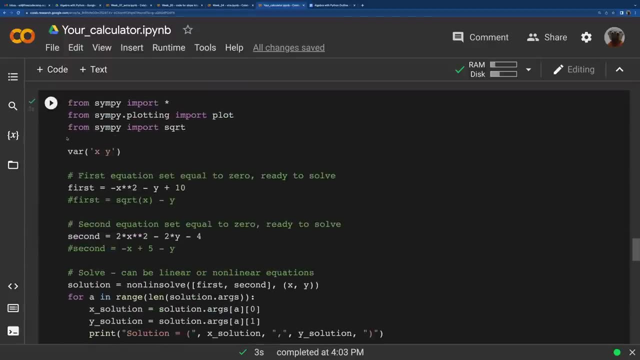 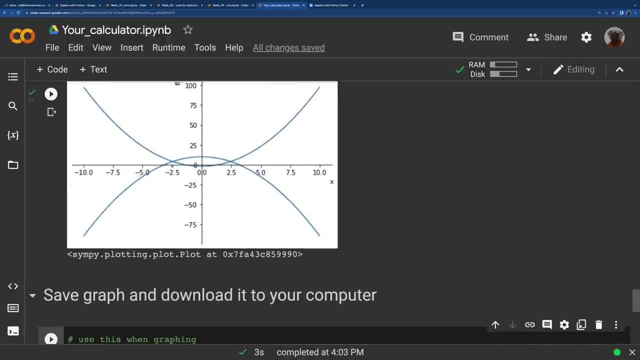 output, because sometimes you might have have something that you wanted to save. So therefore, you take this and you would put, if you wanted to, up here, you'd import that And then, and then definitely you know, you would just do. 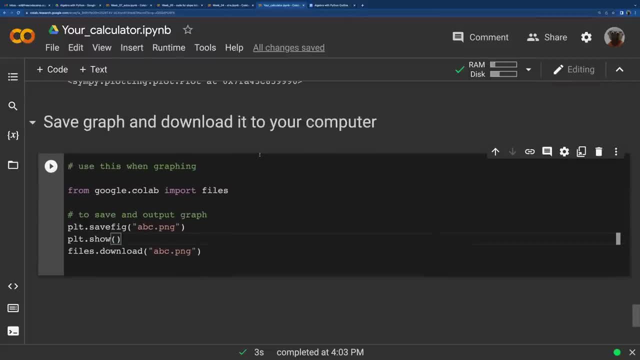 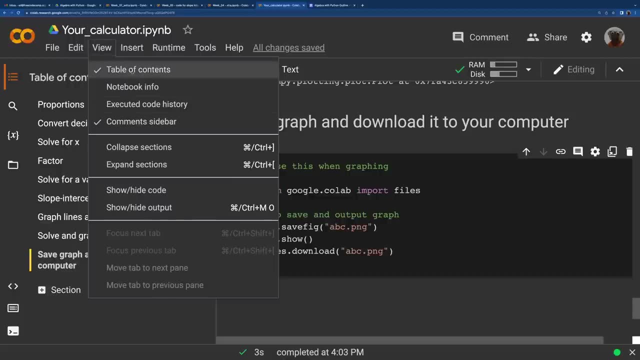 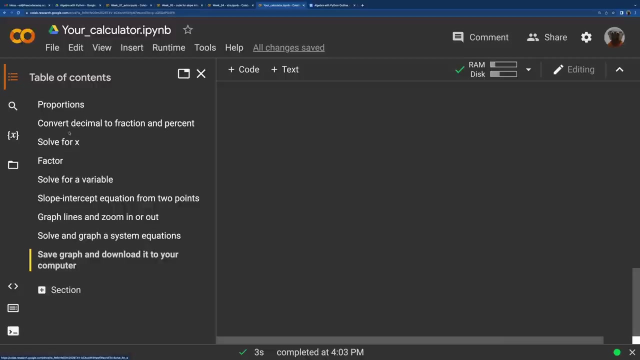 um, save, fig and files download. So there we go, And we have this. now we have all of this And one of the things you can do is, in the view you can collapse all the sections, All right, And now you have all these in your table of contents and you can just jump to them. 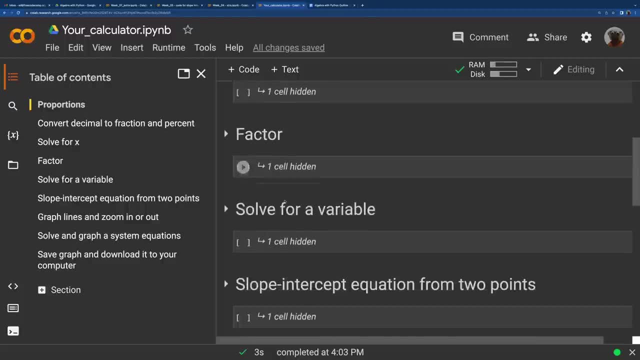 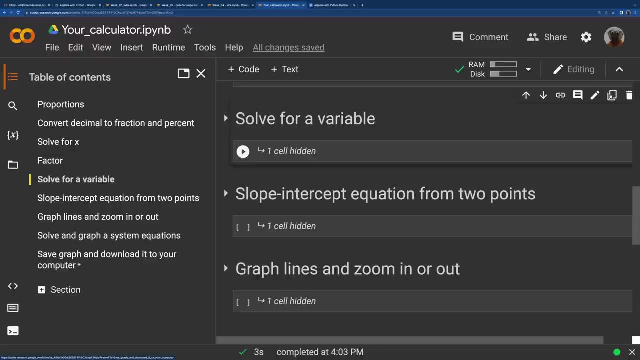 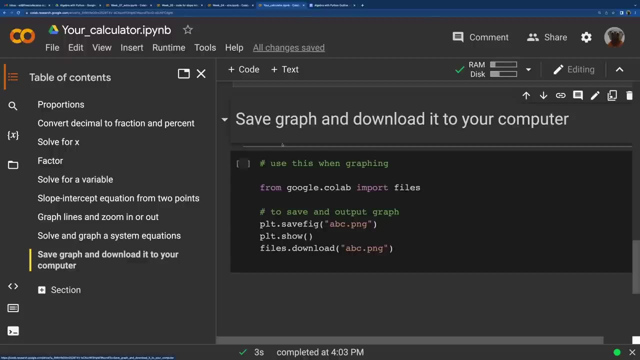 if you need to, There you go. You have all the sections collapsed. and Oh, do I need to solve for X? Do I need to solve for variable? You know, um, I, I like, I like shorter uh headings, so I might and down, save graph and. 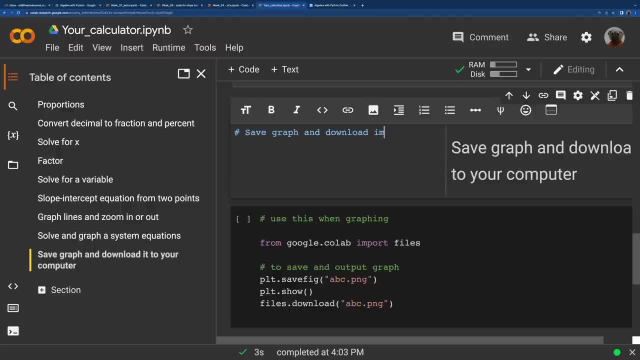 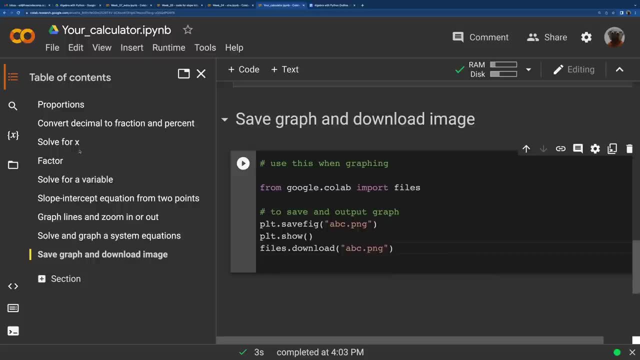 download it. There we go, Cause that's what it does, is it downloads an image. So we're already, we have so much of the core algebra that you're able to do, And you and you can write the code for it. And now you have this at the ready. 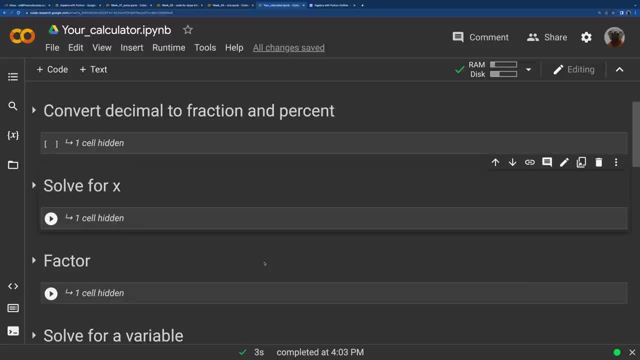 So one of the next things we're going to do is get to quadratics and more complicated graphs. Um, we've kind of hinted at that last one. you know you might if you haven't seen a lot of these- and you say, Oh, wow, Okay, Now this graph has a curve, Now it's getting interesting. 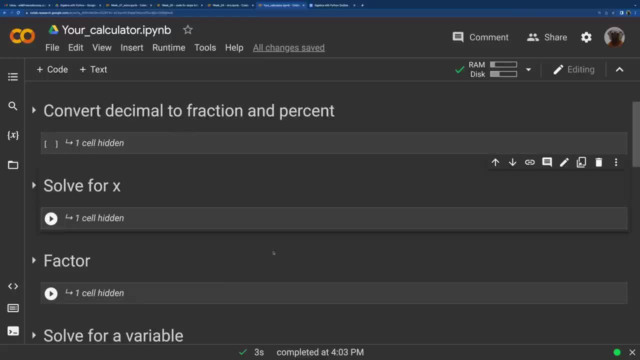 So we'll get into quadratics, parabolas, you know where all the graphs do have a curve to them, and things beyond that. So we'll get into quadratics, parabolas, you know where all the graphs do have a curve to them, and things beyond that. 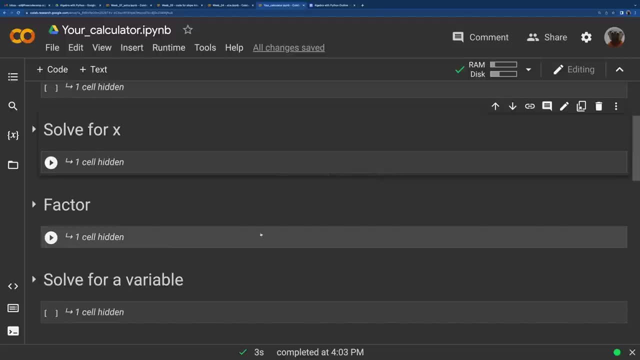 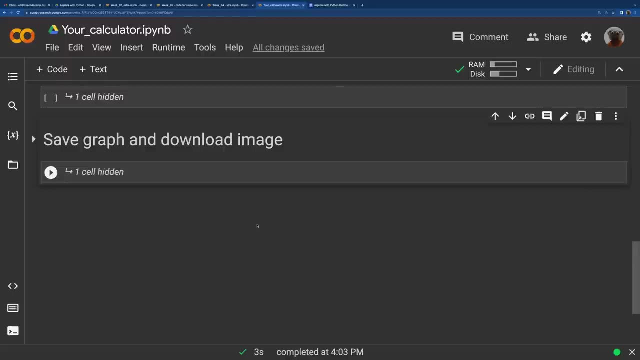 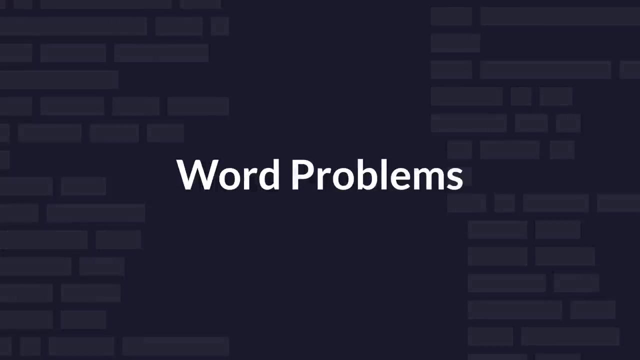 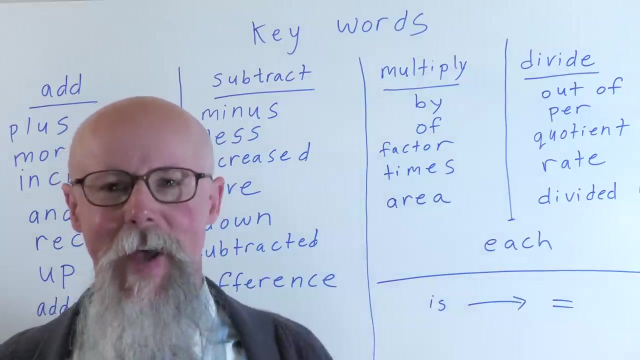 So we'll add more to this, All right, But well, well, on your way to being able being able to solve a lot of algebra problems in Python. So when working with word problems- not just here's a math formula- solve it. 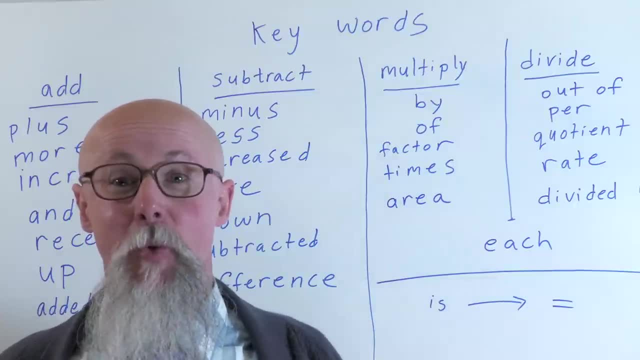 working with you know word problems, or some people call them story problems. working with you know word problems, or some people call them story problems. That's when a lot of times people have trouble translating that into a math equation and we can. 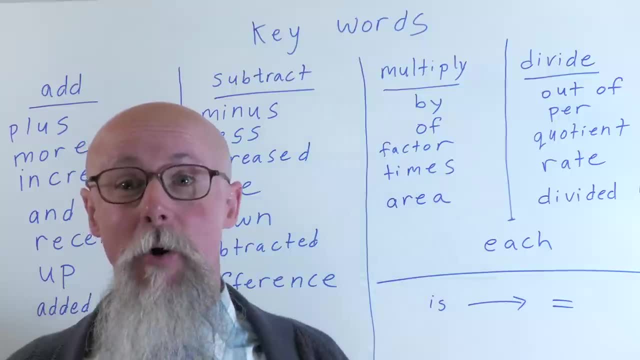 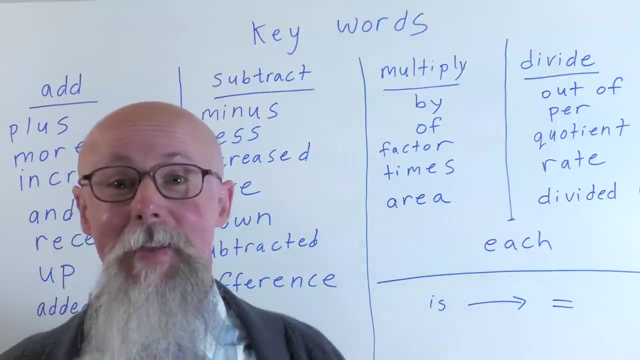 solve. So what I want to do is help you with some key words that you can find In the word problems, in the sentences that have Tell you what math operation to use, And this is not all of them, but this is a lot of the main ones, And 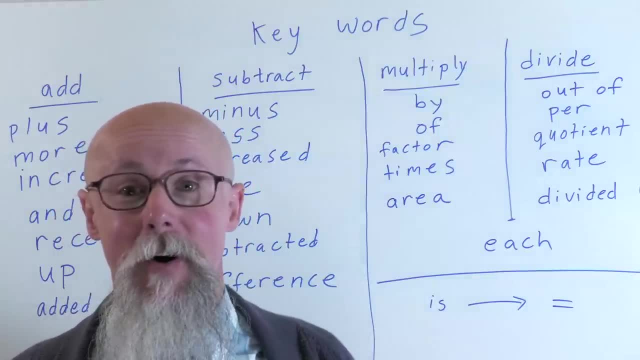 you know you, you get the trend with, So it lets you kitchen, nonsescaped it, and nobody really come for it with this. These are the things that you're looking for, While sometimes, yeah, ask a question, but it's nowhere near where you're going to find this. 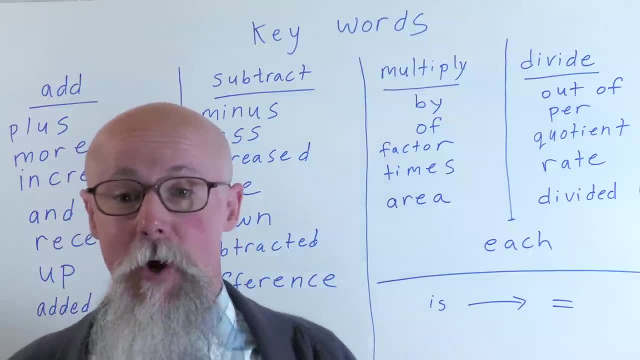 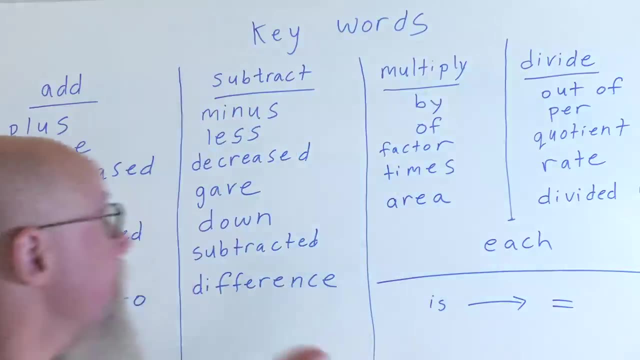 And then, after we look at these keywords, we'll go through a bunch of examples and the code and how to use these translating sentences into math equations. But let's take a look at these keywords. So how do I know if I'm going to add? Well, some of the words are going to. 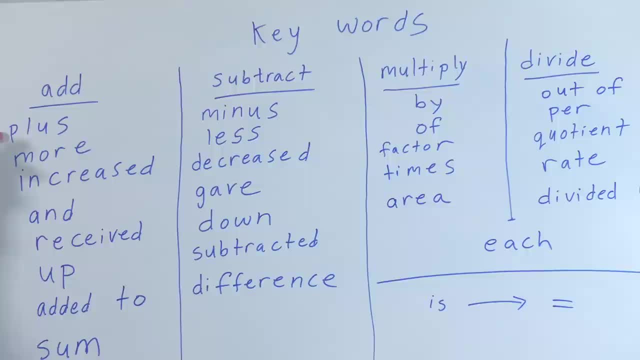 be if I just actually see plus some number, plus another number, more. So if I have something and then I got more, how much do I have now The amount of money I had increased? it might even just be, and I have these cards and those cards. How many cards do I have received? Because a lot. 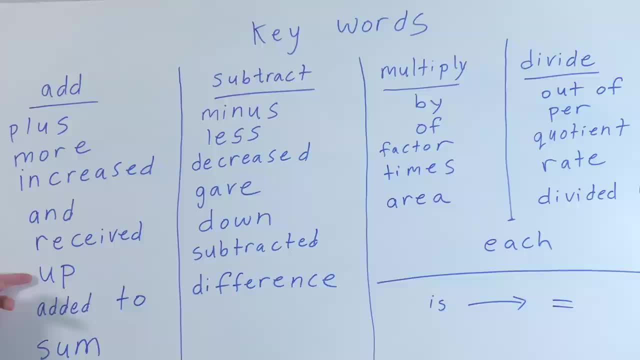 of times that's something added to what we have Up, something goes up, And a lot of times calculating elevation up, we're adding. It might even just come up and say added to Some also, And some means the total when I add up, So we might see some. we might see these, you know. 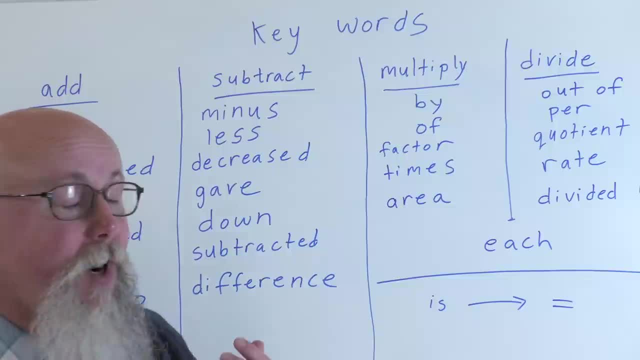 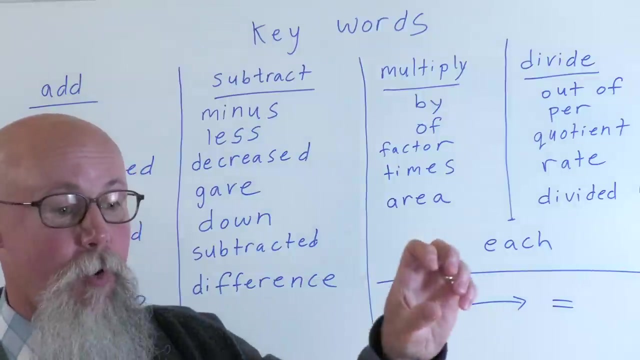 the sum of three and four means I'm going to do three plus four. So these are some of the ones. if you're looking and you see these, then you know you're adding Okay And a lot of this. it's not so exact that you could write a program to find a number, find one of these keywords. 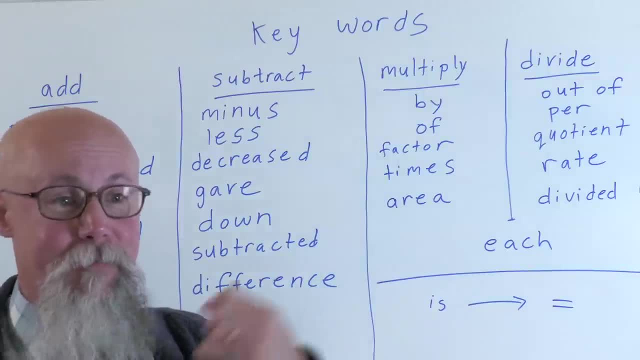 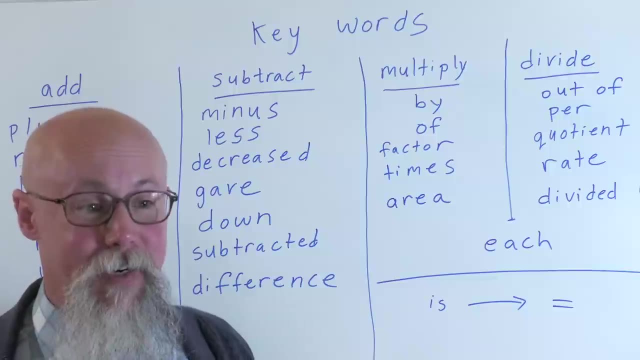 and then automatically translate it to a math equation. So you have to use a little bit of your human intuition there, But it's very much in that direction. You see, these numbers, what, which one of these words are around there, and that's going to give you an indication of the 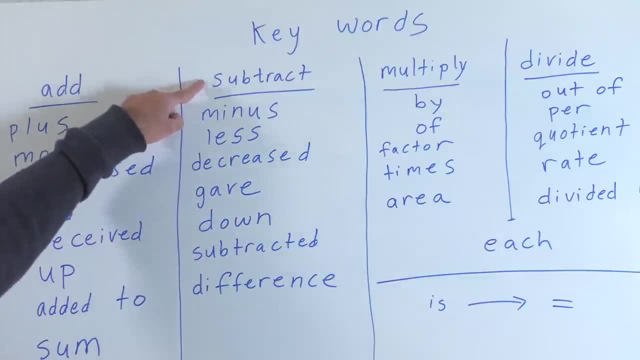 math operation. So let's take a look at subtraction. So subtract, yeah, it might just say minus less. anytime I have less than I'm subtracting, or it decreased, the amount of money in my bank decreased, So I subtract gave, because a lot of times things if I receive something, 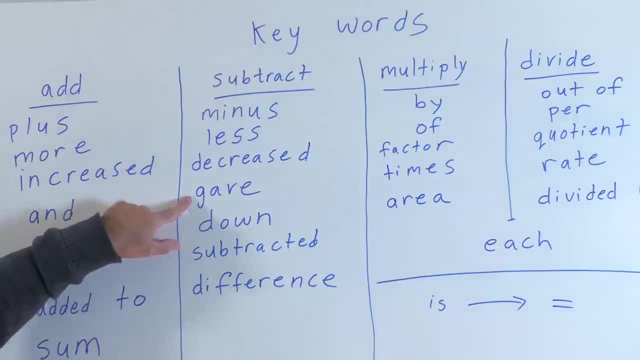 it becomes added to what I have, or if I gave, then it becomes subtracted from what I have down, And that also goes again with looking at elevation. It might even just come out and say subtracted, And then anytime it says the word difference, or I know, I want to find the difference. 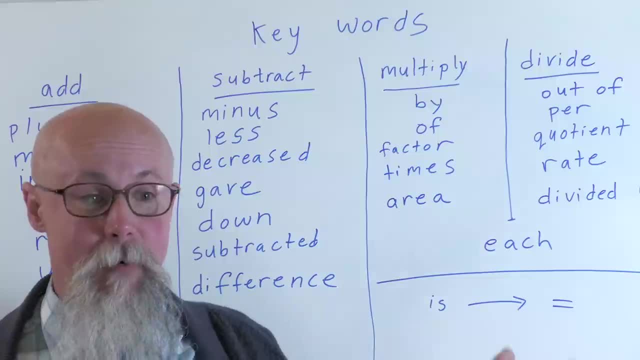 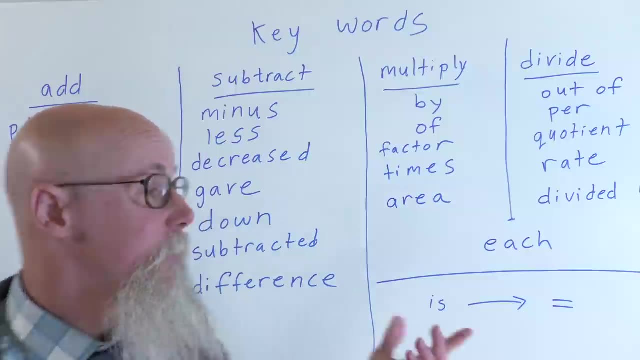 between two numbers. that's subtraction. You know we just find the difference And you know that might be a negative difference, might be a positive, might be absolute value. But if I, if it says difference, or if I want to find the difference between two numbers, 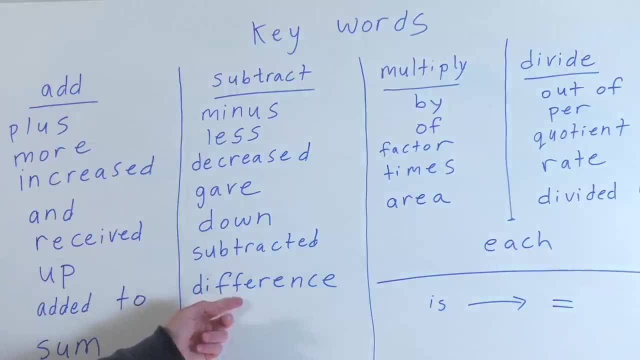 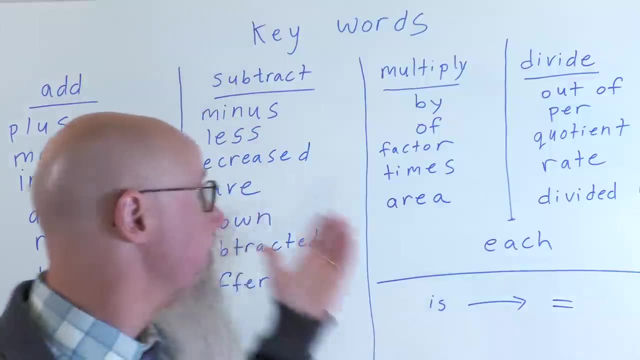 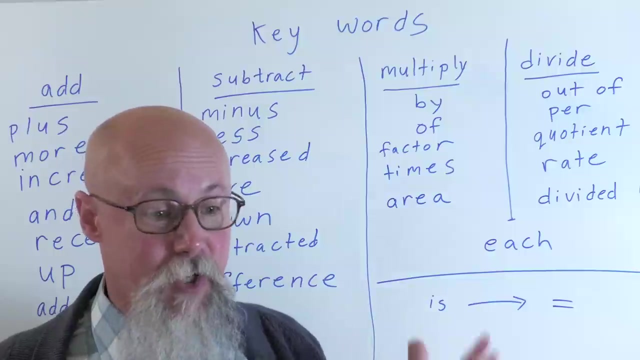 I want to find the difference, then I'm going to subtract, All right, So with multiply. so how do I know that I'm multiplying? Obviously, things are increasing, Like there are, you know. we want to look for that general trend. Things are increasing, And just right away, if you have. 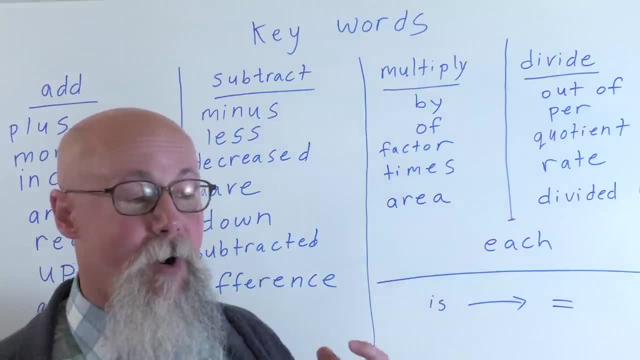 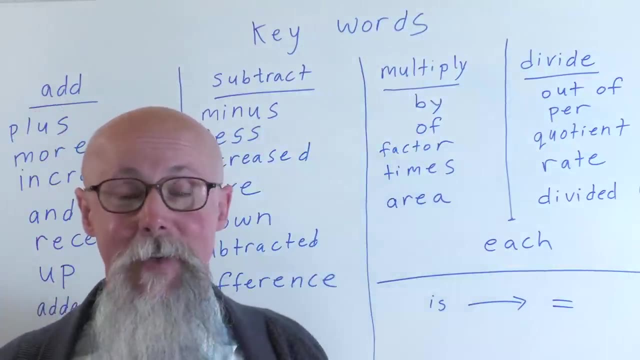 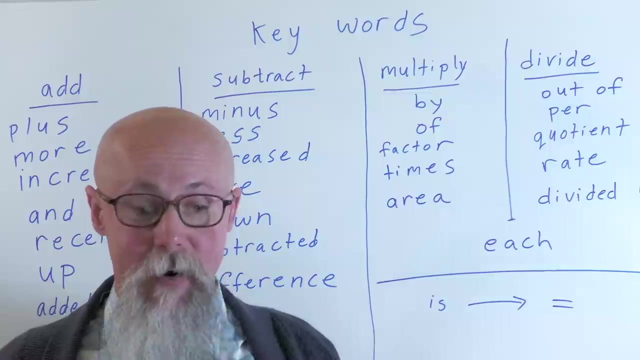 that sense things are increasing. you know it's multiplying or adding. So how do I know that it would be multiplying By just the word by? because if I'm calculating an area of something and then I've you know also then just seeing the word area, but three by five means the area. 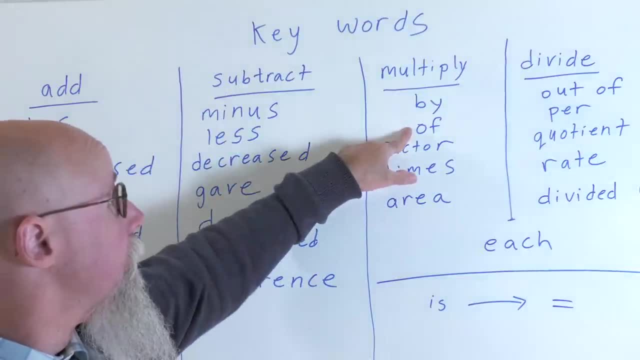 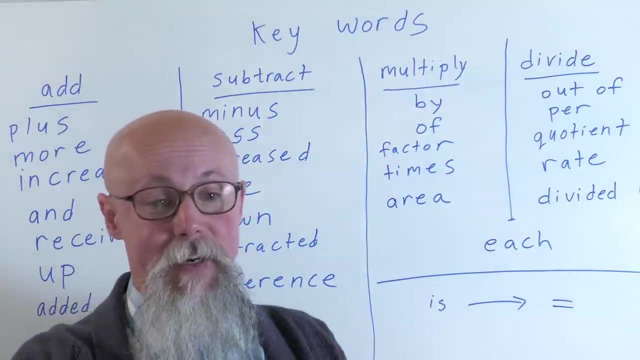 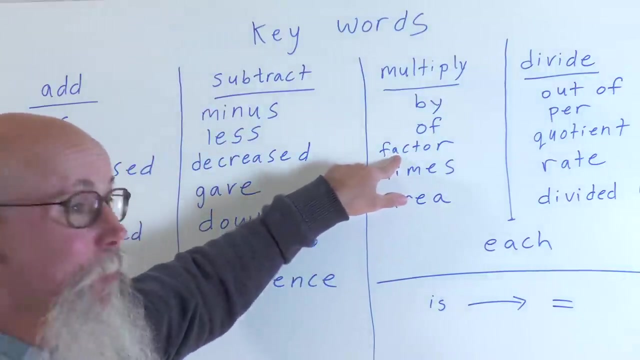 would be three times five Of. so just the word of is going to be: multiply Percent of something. you have the percent and then you multiply times, whatever that something is Factor, because two things that you multiply together are factors, Times. so, yeah, three times. 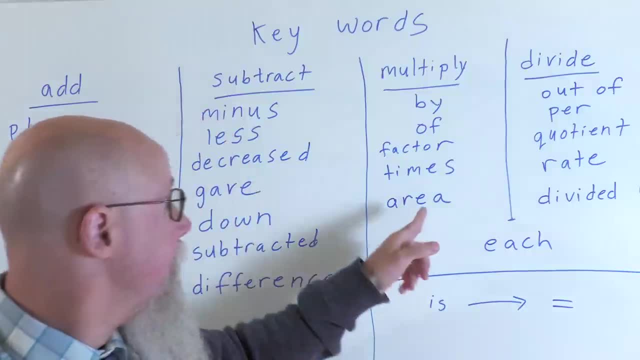 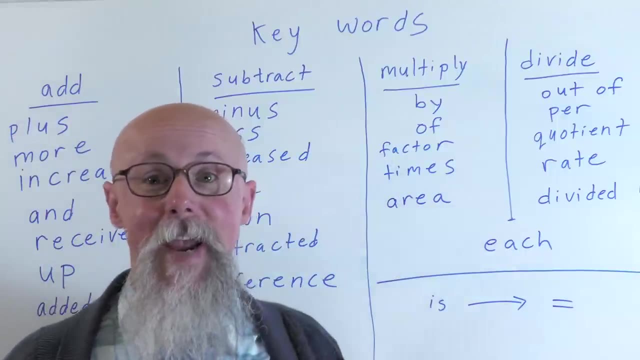 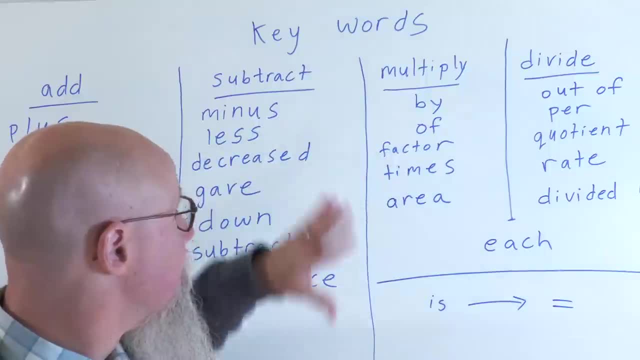 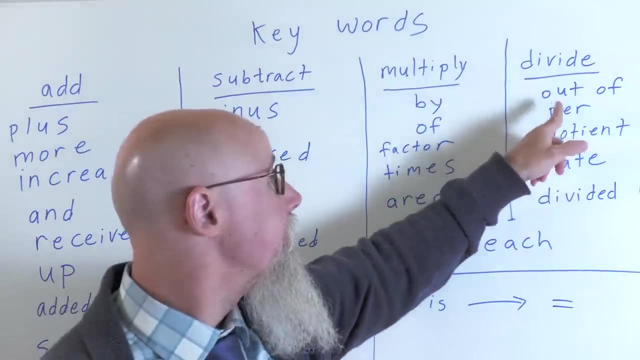 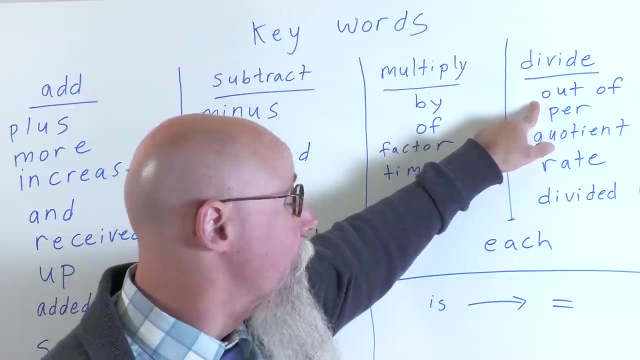 multiplying. So there we go Again. not this is not all the numbers that lead to multiply, but this is a lot of the main one. All right, So divide out of. so notice of would be multiplying, but out of is divide, So you know. 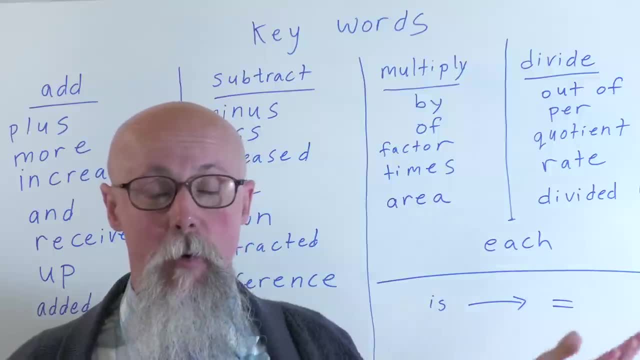 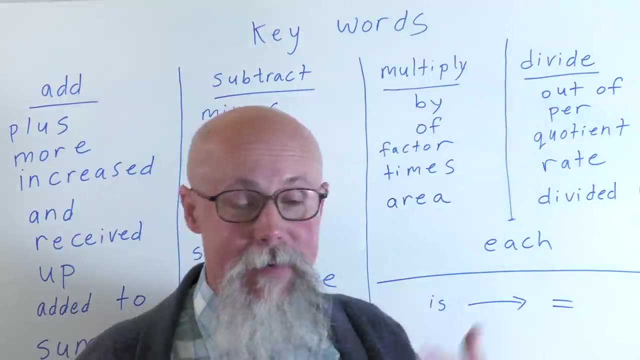 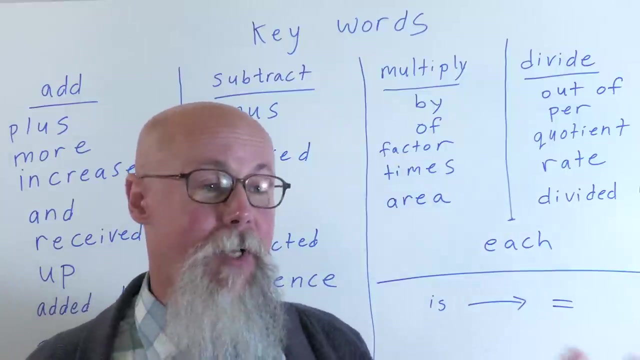 four out of five, that would be a fraction. four divided by five, Per same. actually per pretty much means out of. but that's another way to think about dividing Miles per hour. I would divide miles divided by hours or kilometers per hour. kilometers divided by hours: Quotient? we don't. 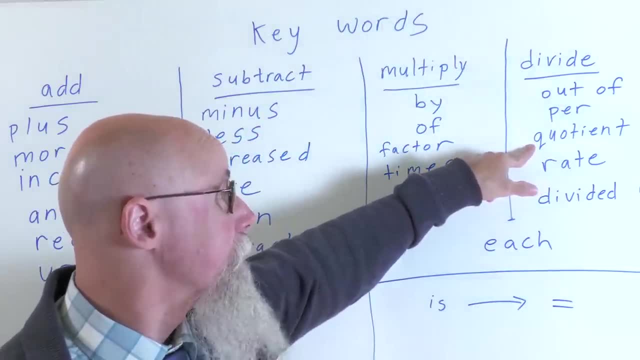 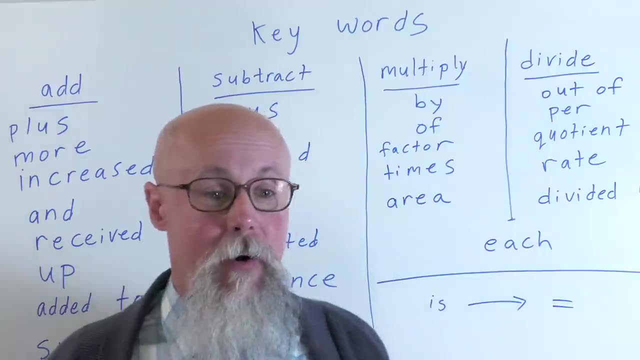 see this word that often, but that quotient means that I'm quotient, the word means that I'm dividing, And actually that's the answer. when I divide, Um any rate, and as I was saying, you know, you know kilometers per hour or something like that. 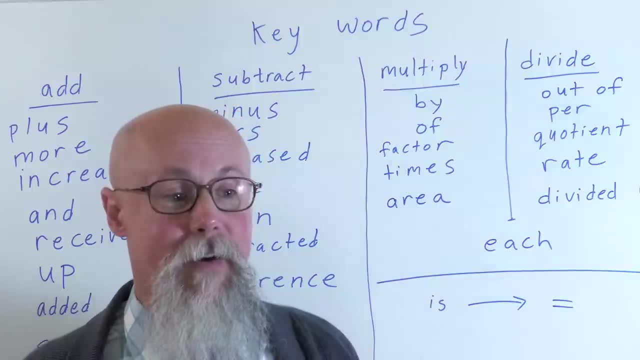 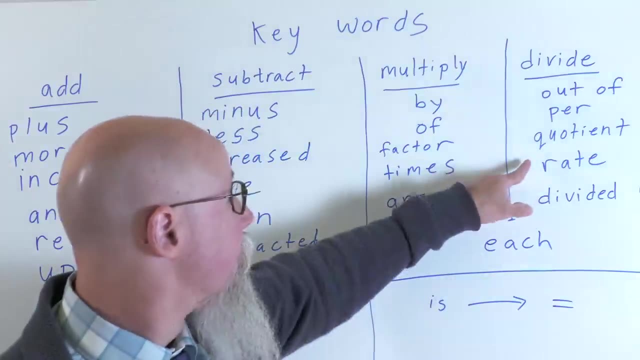 But anytime I have a rate it's going to be some sort of dividing something. divided by something else, uh, usually divided by something related to time, but it's not always So. anytime I have a rate I know I'm dividing something And again it might just come out and say: divided by 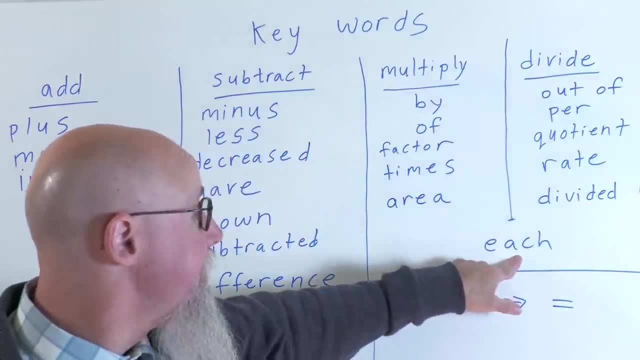 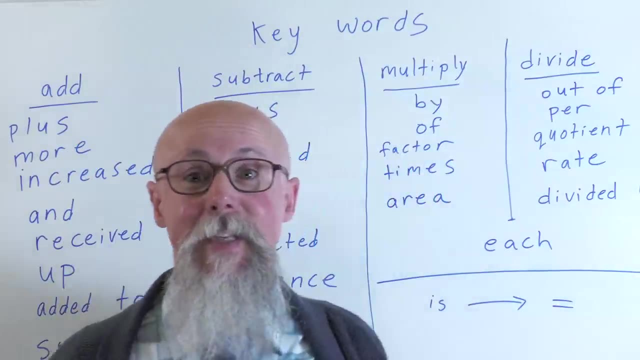 So you know some of the key words here. Now I put the word each here because that actually could be used for multiply or divide, Um, it's the sense of it. You know if I have um, if I have 20. 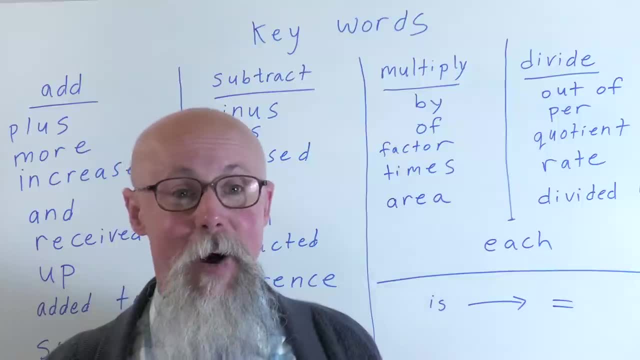 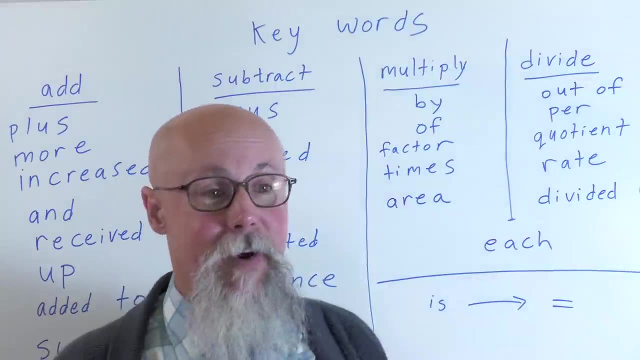 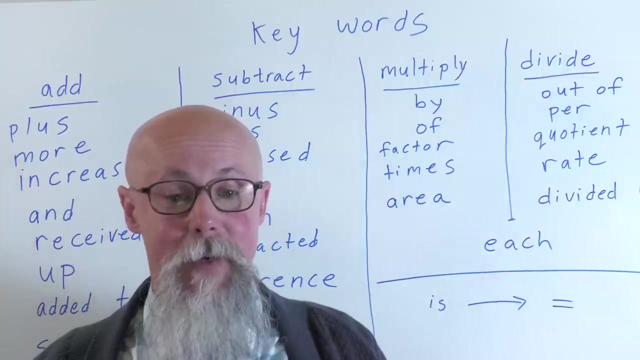 students in the class and I want to give them two pencils each. how many pencils do I need? So then that's multiplying, because I have to do 20 times too. But if I have, if I know how many pencils I have, and then you know, I know, and then I have 20 students and I, you know how many. 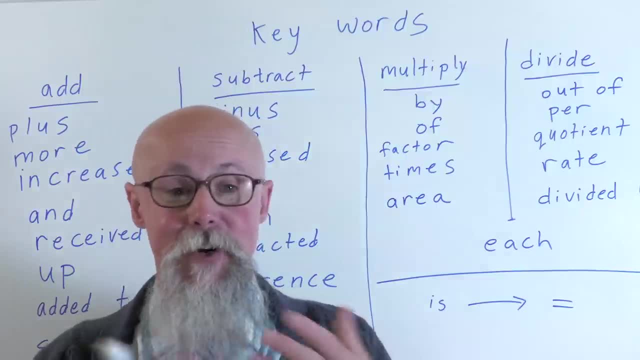 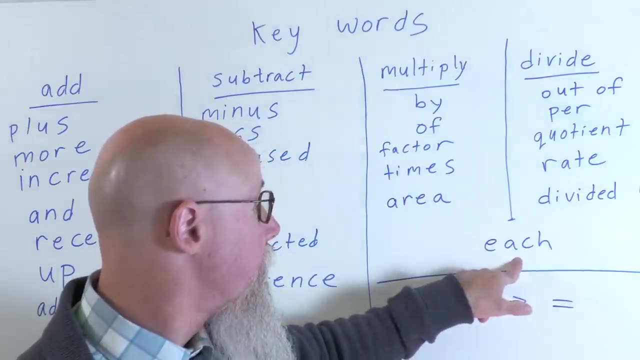 can I? how many can each of them get? Yeah, You know, if I already know that I have 20 and then I have 20 students, how many can each of them get? I'm dividing, So each can go either way. We have to get the. 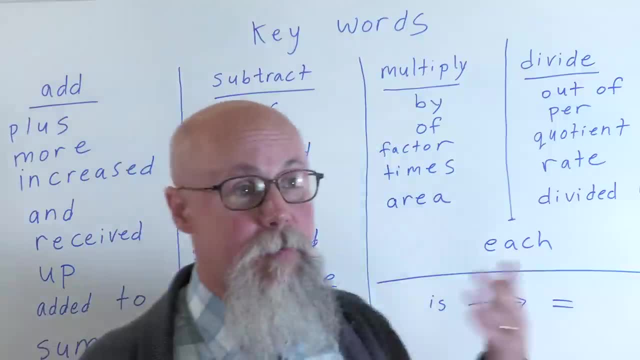 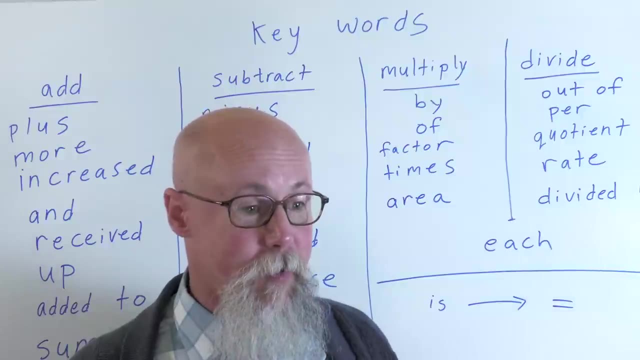 sense of it and dividing like subtraction. If I get the sense that it's getting to be a smaller number, that I know it's dividing or subtracting, you know, and then we, we can look further. you know what's the sense of it? Am I, is it something you know, each you know. 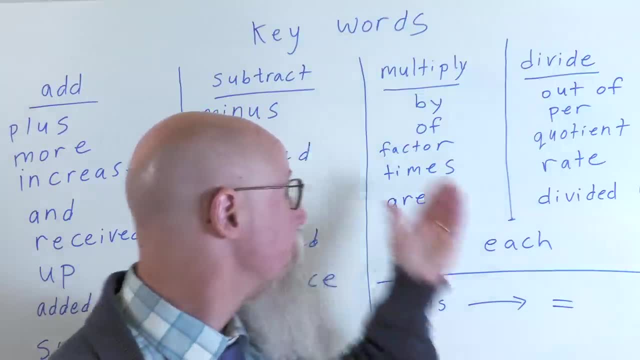 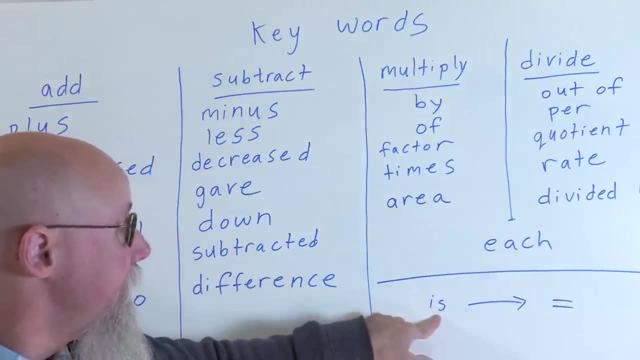 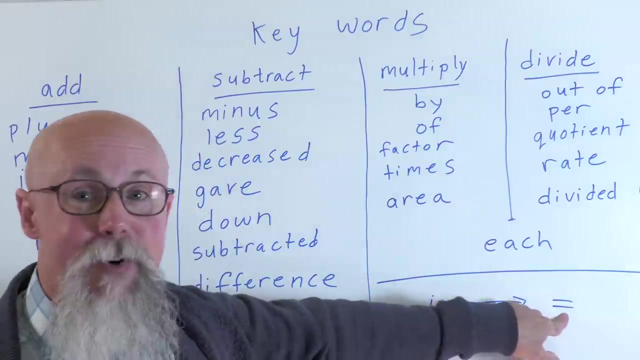 I'm dividing it out among different things, or is it just a subtraction, Right, Okay? So these are some of the main things, And the one that carries over a lot is, or some version of is, are, was, but is translates to equals, So that's where we get. 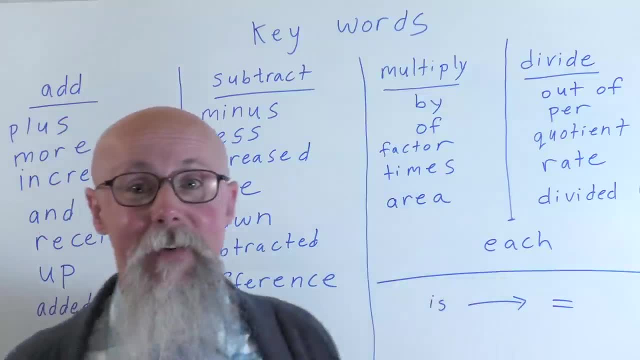 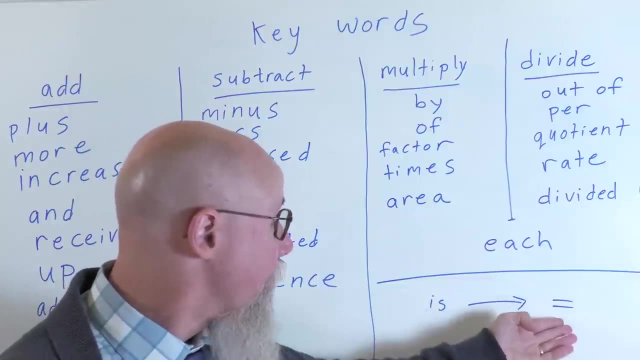 the equal sign coming into our equation And so if I have these then I can translate. you know this is, was, will be something like that becomes the equal sign. So, looking at these keywords, you know we get the numbers from the, from 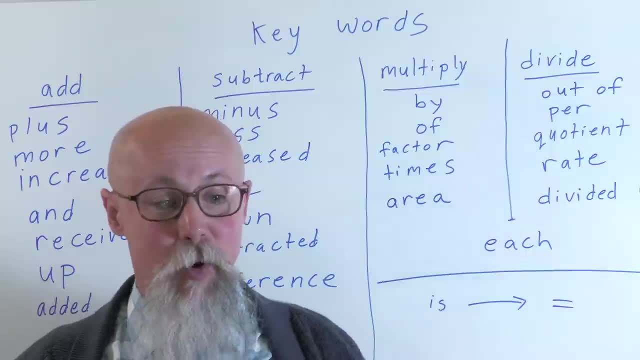 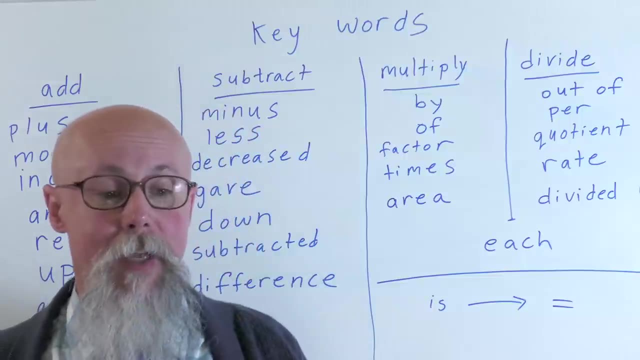 the situation, as well as these keywords, and we can put together an equation, And so I wanted to give you these keywords and then, in the code, what we're going to do is we're going to look at a lot of some sentences and translating them into math equations and 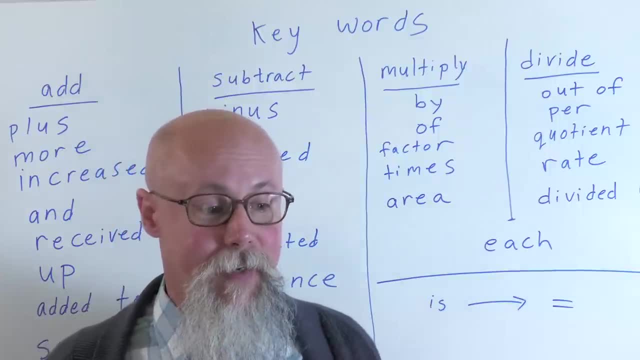 then, of course, solving them. But that's what we want to do. We want to be able to translate this. You're not always in life going to have like: here's the math problem. It's going to be some words and we have to translate that to a math problem. 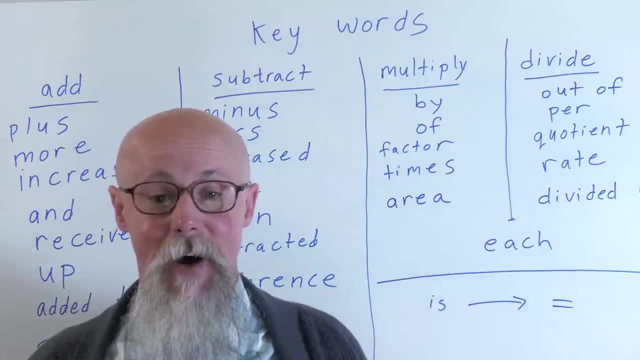 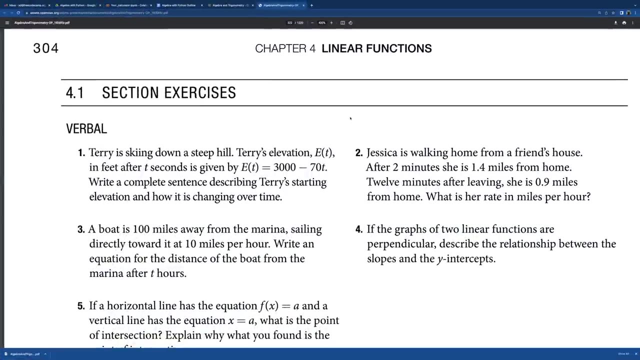 So let's take a look at how to do this. Let's apply these. translate some sentences into math problems, All right. so let's take a look at the code. So now let's put some of this into practice. Some of the math we've been talking about with the linear equations, slope, intercept. 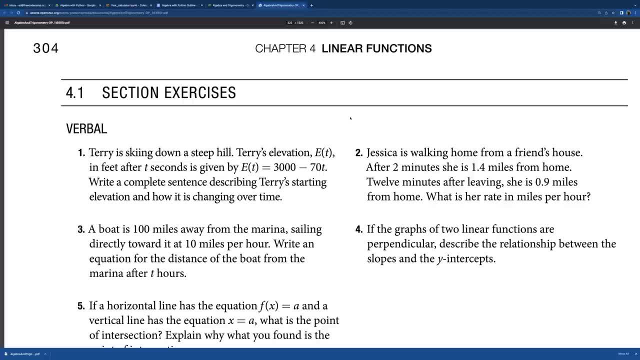 especially, and some of the Python developing equations, finding slope graphing, all that. Let's put all this together and use that to solve some problems here. And first let's look at how we can see That y equals mx plus b. pattern for a linear equation show up in slightly different ways. 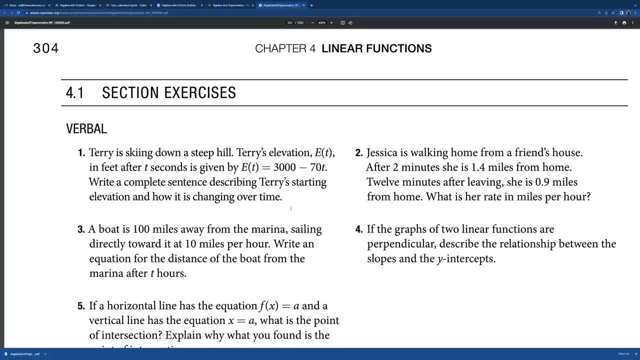 You know, sometimes we just change out the letters a little bit, but be able to recognize that pattern. So if we take a look at number one- and this all comes from the textbook, the one that I have listed as textbook two- algebra and trig. 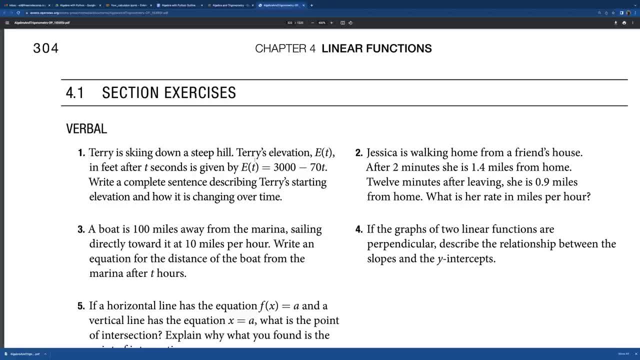 So you know, there we go, Page 304. You can find it, Find these. I'm just going to pick a few of these and I want to highlight, you know, what we can do with these. So if we take a look, Terry is skiing down a steep hill. 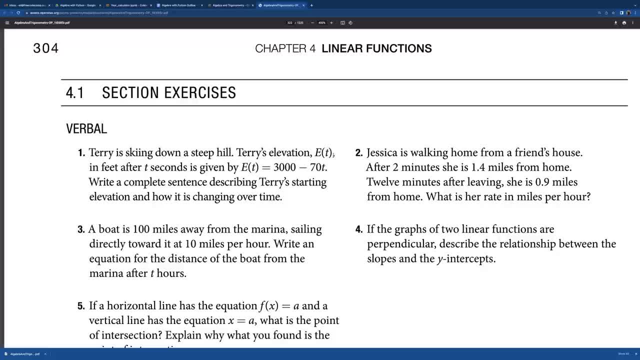 Terry's elevation e of t. that's how I'd write that. That's the function, instead of just y equals. we'll call it e of t. elevation as a function of time. Terry's elevation in feet after t seconds is given by this: 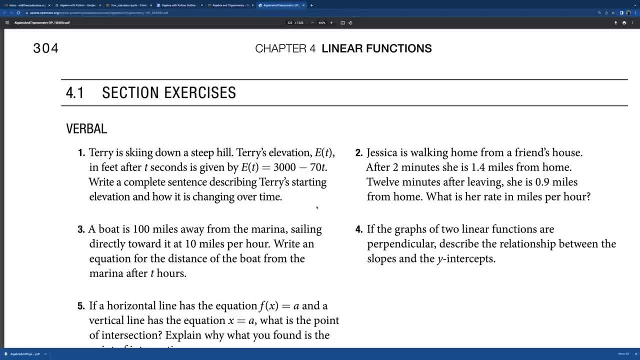 So e of t equals 3000 minus t. That's the function. And we see then. you know, instead of x we're using t because it's time, And we have 3000 minus 70 t, And then our y value is e of t. 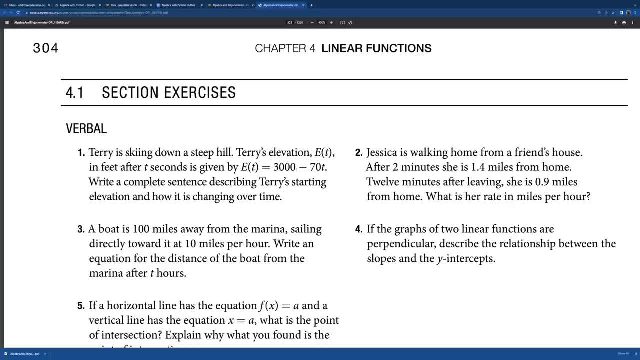 That's the function. And so we see the slope. the intercept come first. That's where we begin. She, uh, Terry begins at 3000 feet up and then goes down the slope at 70 feet per second. So we see the slope. the intercept come first. 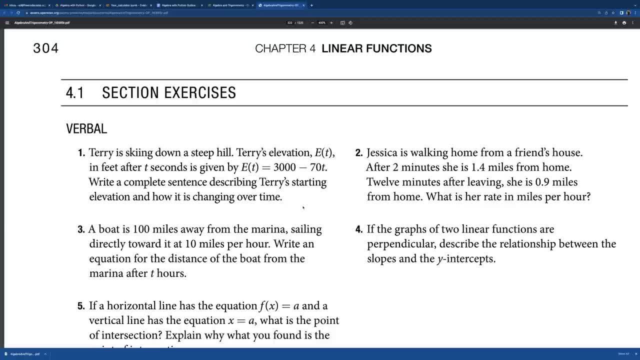 That's where we begin. She, uh, Terry, begins at 3000 feet up and then goes down the slope at 70 feet per second. So we see that that is the slope, the slope of our equation on the slope, and negative because that elevation is going down. 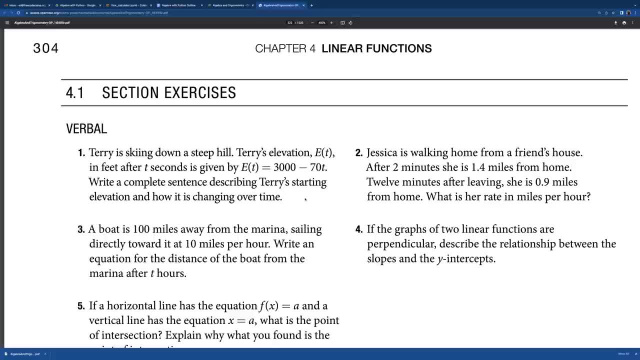 Um, there we go, So we can see the slope. We can see where Terry begins, 3000 feet up. Um, and there we go, Just finding that slope. We just look at it and we take a look at number two. 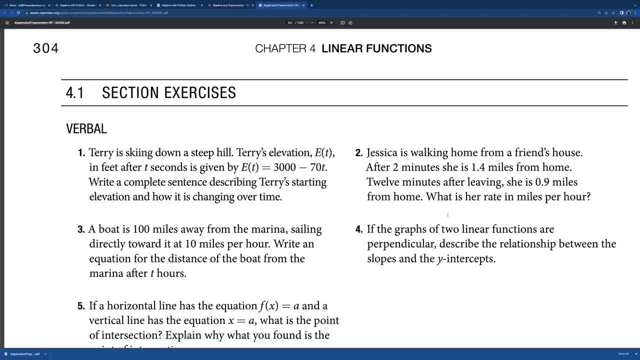 Now we have Jessica walking home from a friend's house. After two minutes, She's 1.4 miles from home. 12 minutes after leaving, she's 0.9 miles from home. What's her rate in miles per hour? 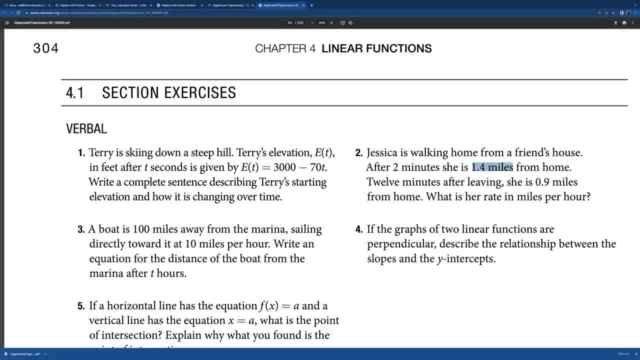 Well, right, here we have distances in miles, but the times in minutes. So if the question asks for miles per hour, we definitely see also that we have two points. We have a time and a distance, and then another time and distance. So we'll you know, X will be time. 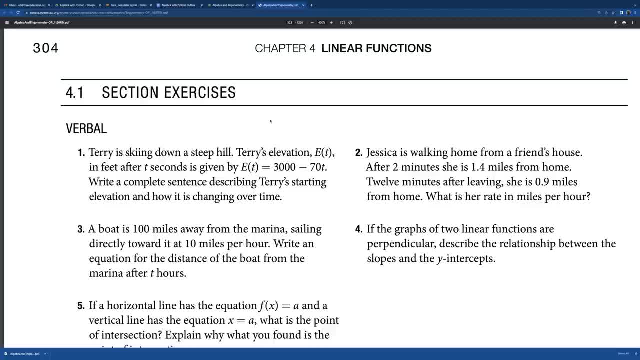 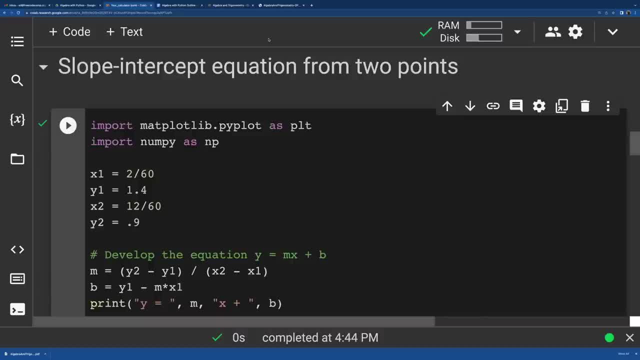 Y will be distance. Okay, And having these two points, we can go to our calculator. Now, hopefully this lines up with something that you've already created. Um, you know, remember we might've called it like your calculator. and then, hopefully, 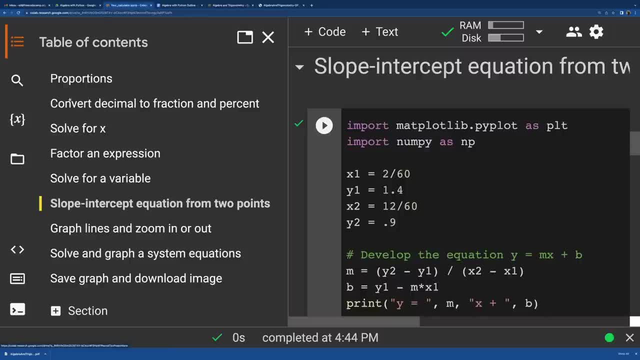 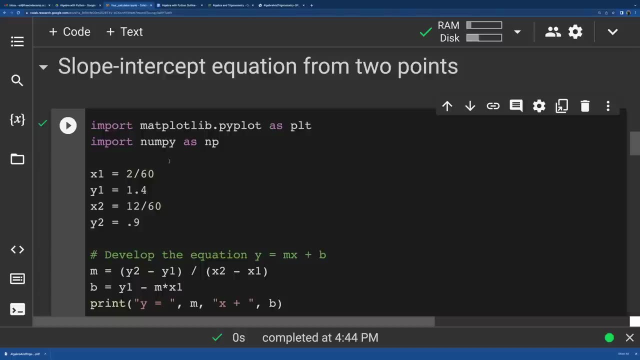 you know, then you would have created the table of contents for the different things that we want to be able to do. And we can jump to here, slope, intercept equation from two points, because even though that question For the full equation and everything we're going to do more, um, but the first thing. 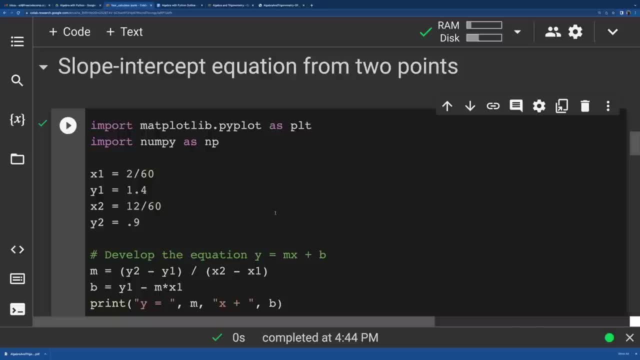 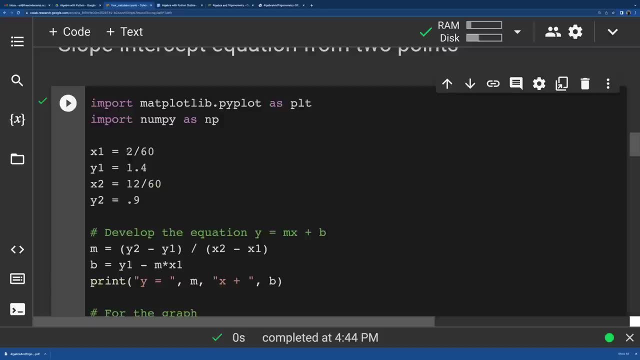 it's going to do is find the slope for us, And hopefully you know that's it. you know we have these formulas, you made these. now we can make use of it. So you would have had all this and then we would just change X1, Y1.. 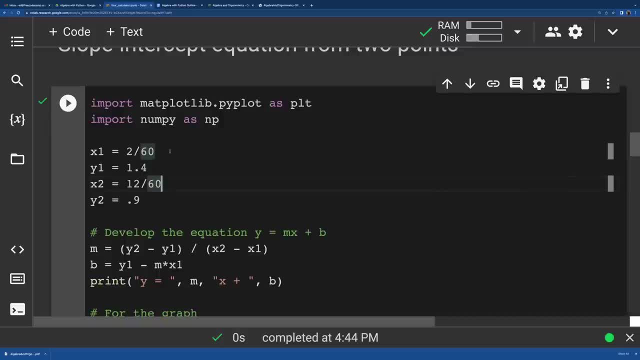 So the Y value is 1.4, but that X value it's two minutes and we have to remember, so I already put this in here. Okay, So it's two minutes and there's 60 minutes in an hour, So it's two out of 60.. 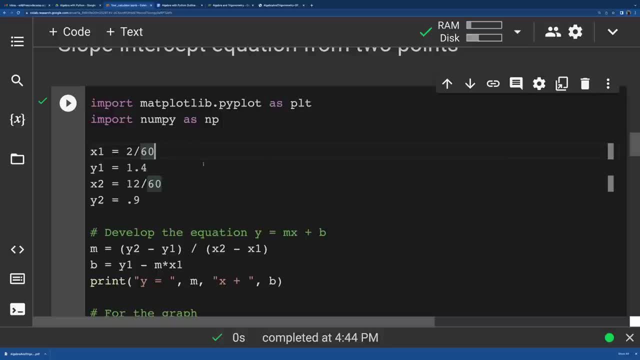 You could reduce this if you want, but you don't even have to. Python will take care of that. in the other, in between steps and the Y value 1.4 miles. So the second X value 12 minutes. So same thing: 12 minutes. we want it in hours. 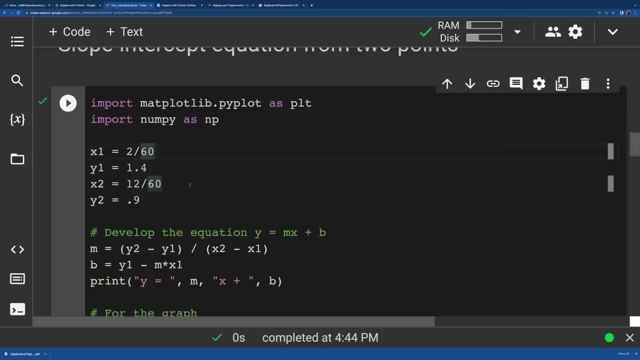 So it's 12 out of 60,, again, that reduces, but you don't, you don't actually have to, And then 0.9.. Okay, So, having all this, you can just put in these four values here, calculate the slope intercept. 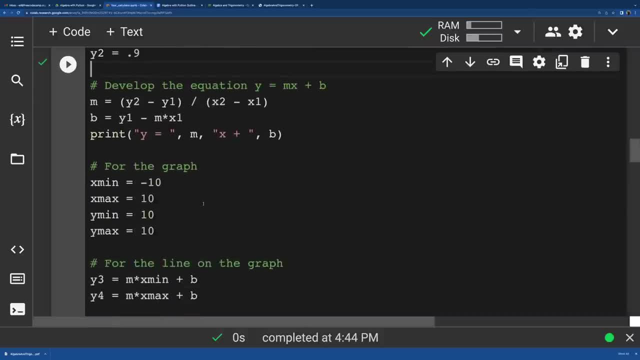 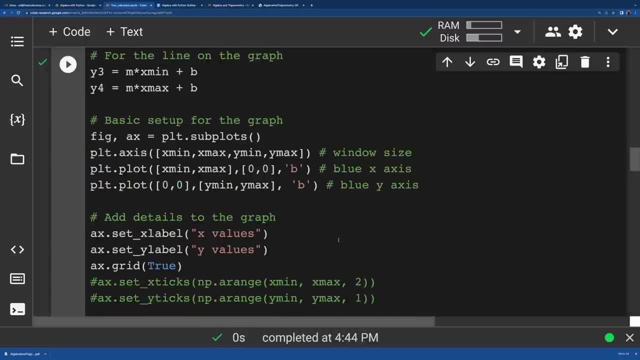 We'll print that out, So you see the equation, and then we'll also graph it. I mean, we're going beyond what the question is, but this will give you an idea of some things you can do. You already have this, And all we needed to do is recognize what these values were, put them in here and then. 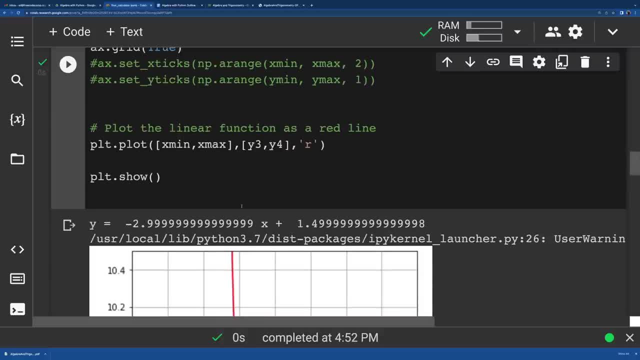 we run it All right, So this Okay. So we would take this slope as three. So sometimes, just the way Python calculates things, it might be this: 0.9999.. It's three, And if you really wanted to seeing this, you know you could always go back and put a round. 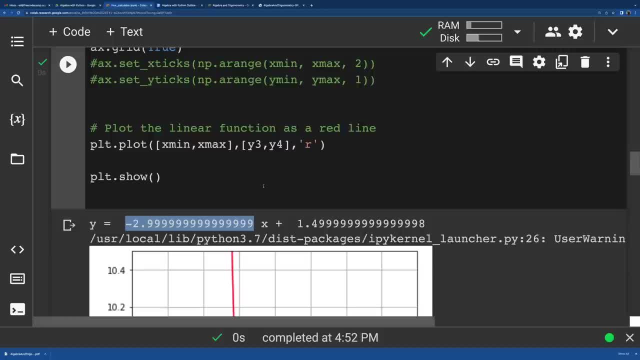 function in in your code. you know, round it Same with this. You could always round it to two decimal place, to one decimal place, which would be 1.5.. Okay, But either way, we see that remember. our first point was two minutes after she left. 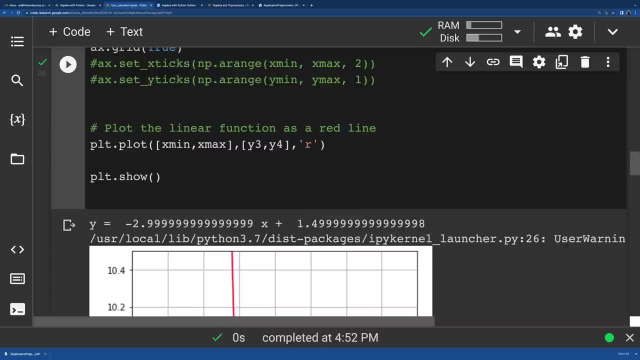 So at time zero, at two minutes, she was 1.4 miles from home, but at time zero she's that little bit more, 1.49 or 1.5 it might round. So we get our values here and you know again, you could put a round function in there. but 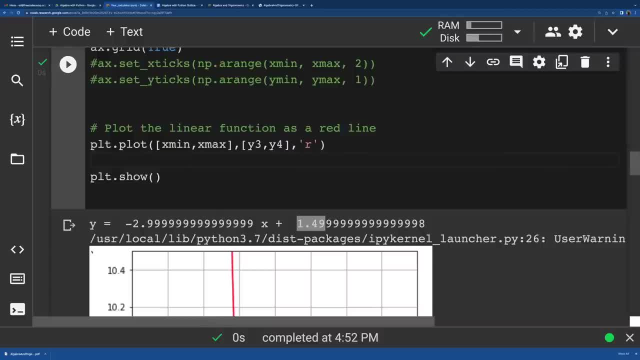 I'm not worried about that right now. And also Python. It gives us this warning, but it's still ran. Occasionally that happens just the the, the way it calculates some things. um, you know, we get, uh, a warning. you know some value, maybe not even related to what we were working. 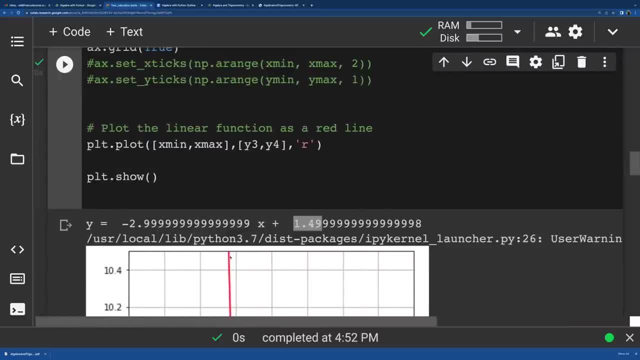 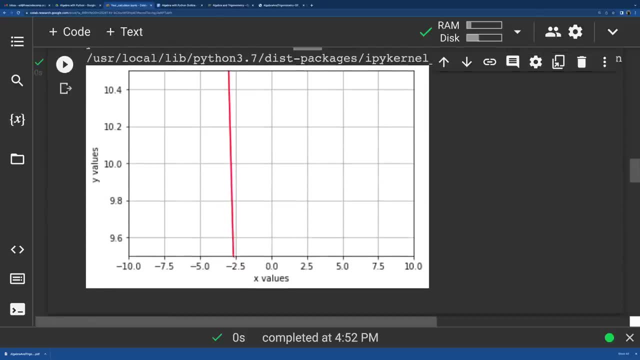 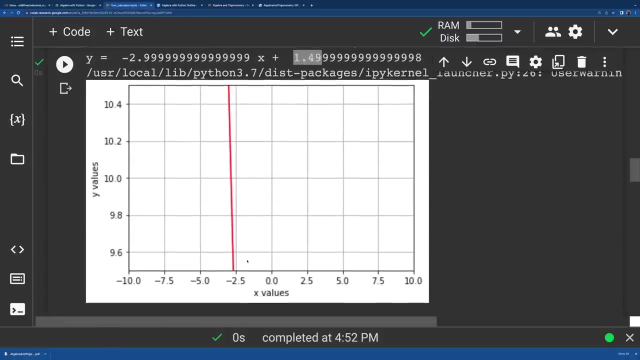 on Um gives us this warning, but it's still ran. It still gave us all this. And then we also have this graph. Now, if we have, you know, the X values or the Y values, So this is her time from home. 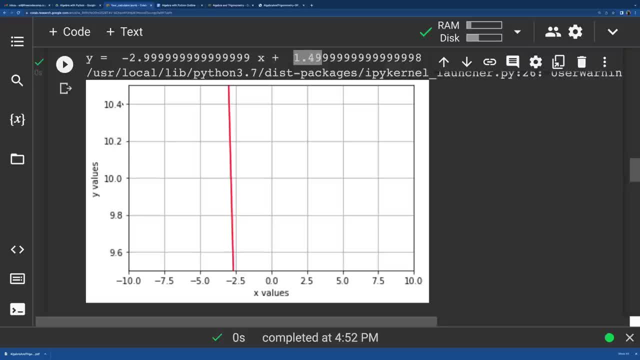 So this Y value- notice, it seems like this graph is completely irrelevant, because the Y value only goes down to net 9.6.. We want it down to zero And then we have negative time values. What do you know? What's that all about? 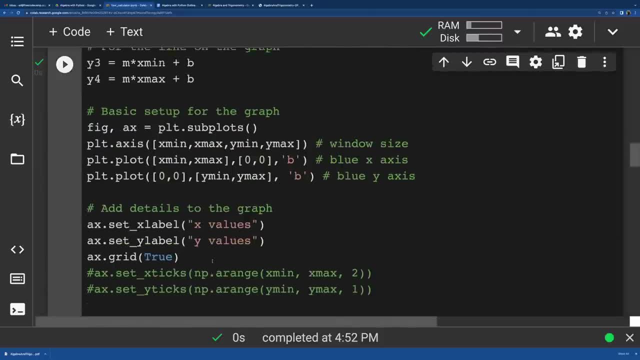 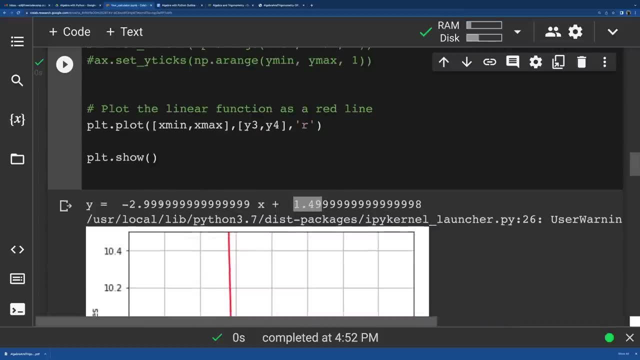 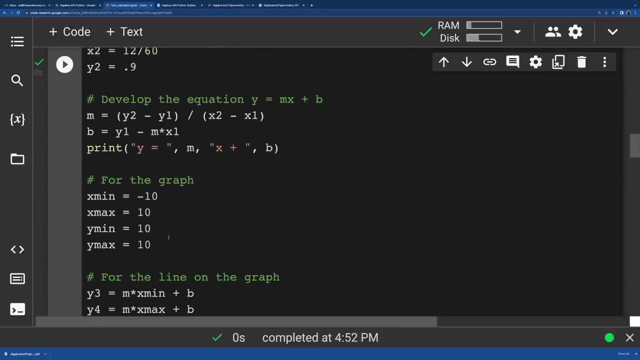 So Remember mathematically a lot. you know all these things already exist. These values exist. You know we make this equation here negative: three X plus 1.5, but that whole equation exists, So we can actually change the graph. 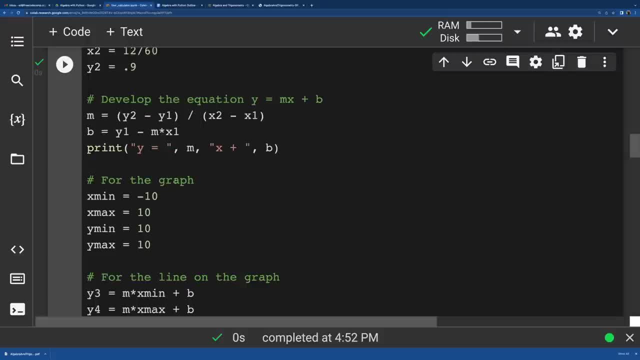 And one of the things we have you know later on in this document is: you know we can graph, you know you can always graph and zoom, but we can just change the graph here and our X minimum, If X is time, we can just make that zero because negative time. you know she was still at. 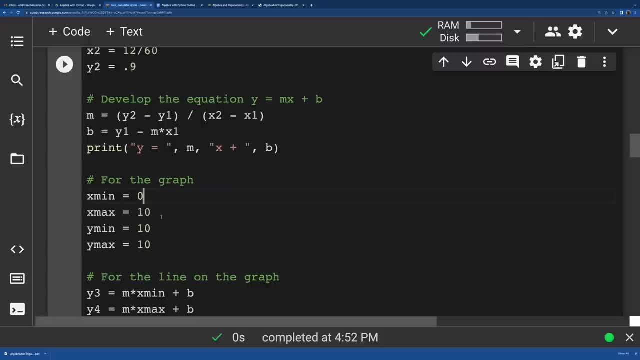 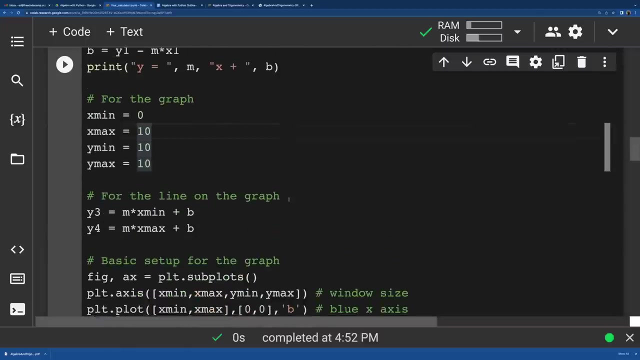 her friend's house, So that won't affect the, the walking and the X maximum. I mean we can really zoom in. Um, now, once we figured out that she was going three miles an hour and she only had half a mile to go, like we can make our X value really small. 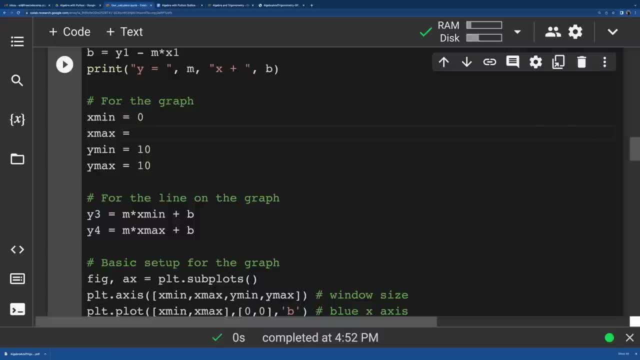 Um, I don't know I'll. I'll reduce it to five for this one, And the Y minimum is zero and the Y maximum I don't even need that to be 10.. Um, I can even make it. I'll make it five, but we don't even need to that much. 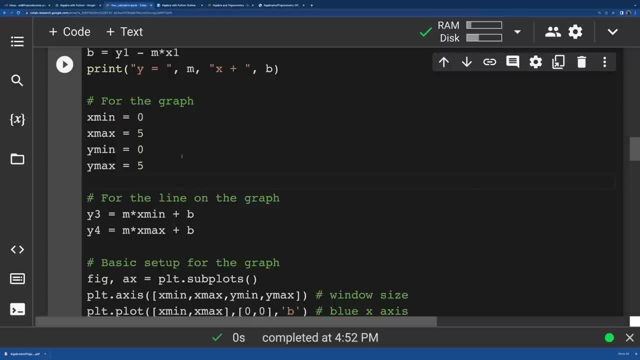 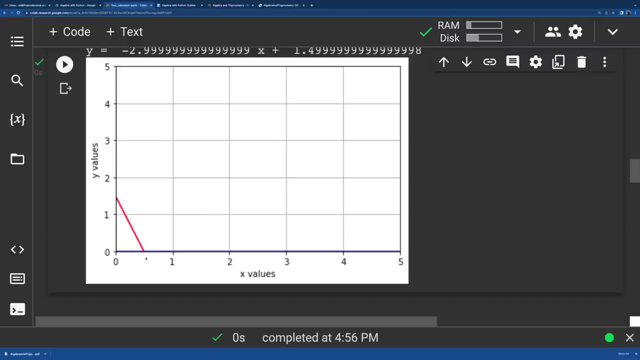 We can really zoom in on this because it's a relatively short distance. All right, So now when we have this, now we have Graph we can zoom in on and you know, this is the only part we needed, So we could look at this that you know, about one and a half miles away. 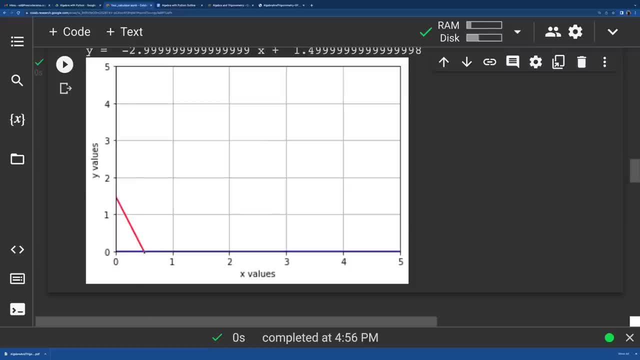 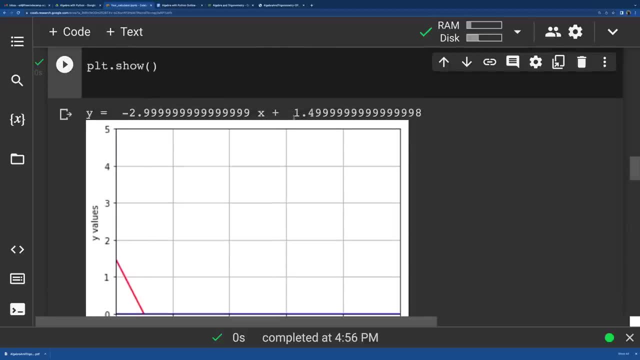 And so, therefore, you know she's walking about three miles an hour. It takes her about a half hour to get home, And there we go. We see, you know the rate, you know the slope, the whole equation. 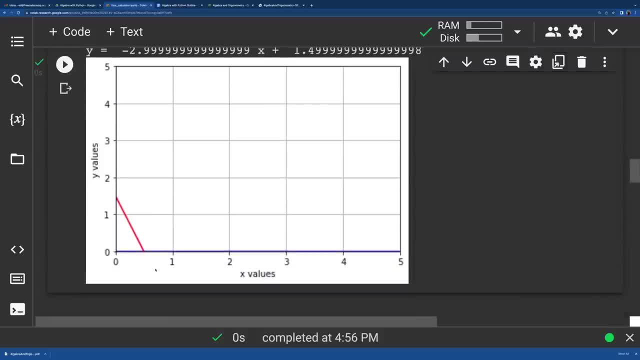 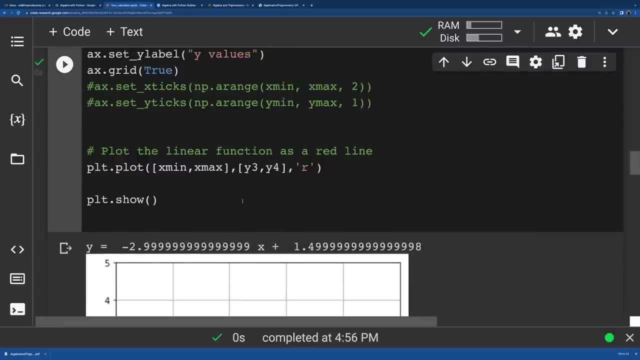 We see, We see the graph, and then we can graph the trip home. We could also always, you know, change these. you know. if you really needed to explain this, you know, to someone else, you could always put, you know, X values. 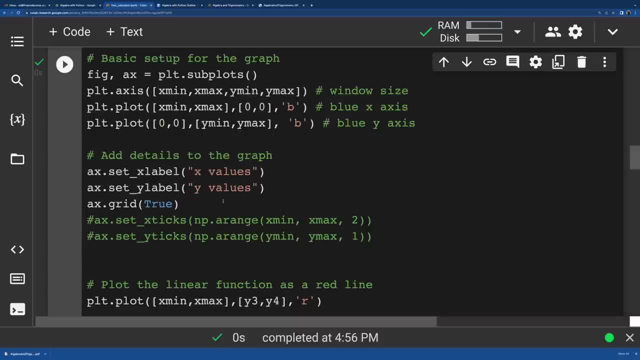 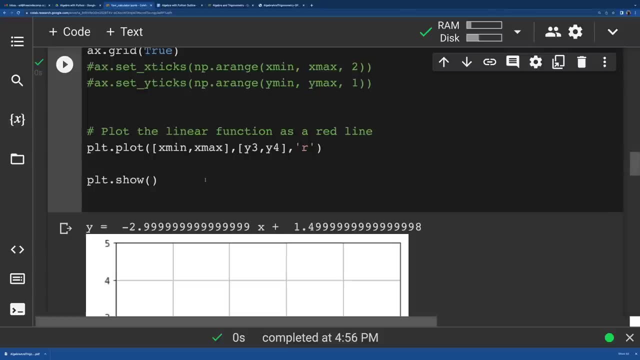 You could change that to time. Y value can make it distance from home. So there we go. So we have these calculators that you know. we're talking about it here. I'm talking about it here a lot now, But if you had this at the ready, 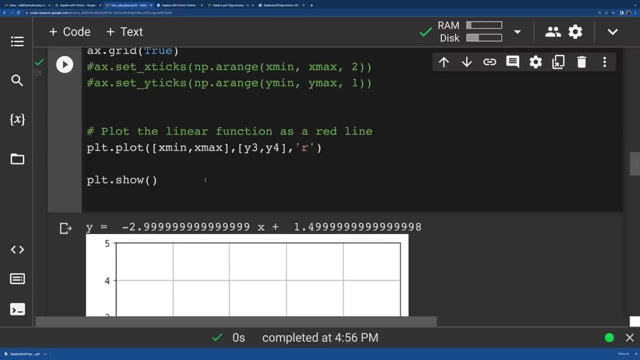 You might even just um, you might, you might even just. you know, see this. oh, I see my two values. plug them in, click run and you have your answer, you know. move on in a few seconds here. 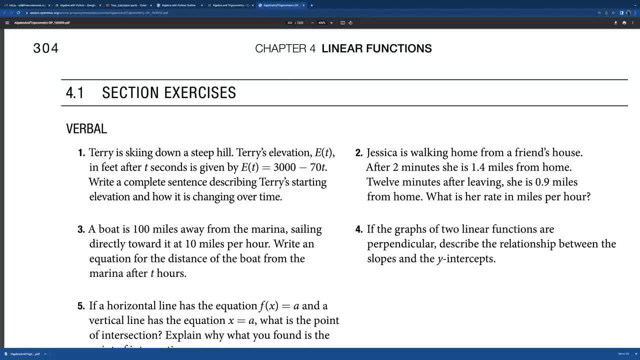 So some things we can do here. um, notice number three, very similar, And maybe we'll do number three. you know, a lot quicker. A boat is a hundred miles from the marina, sailing directly at it at 10 miles per hour. 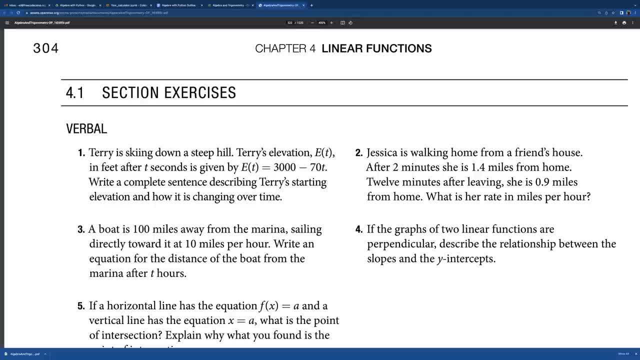 So now we already know that equation because it's a hundred miles away. So that's where we begin, at 10 miles or an hour, And if we want the distance from the marina, then it's a negative 10,, a hundred minus 10 X. 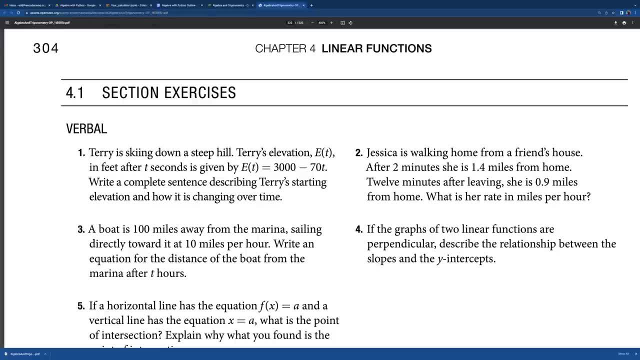 So we could always go here like that's the equation, a hundred minus 10, X, And we could always go to something else and we could graph that, Uh And see, you know just the trend. how long does it? how long will it take for the boat? 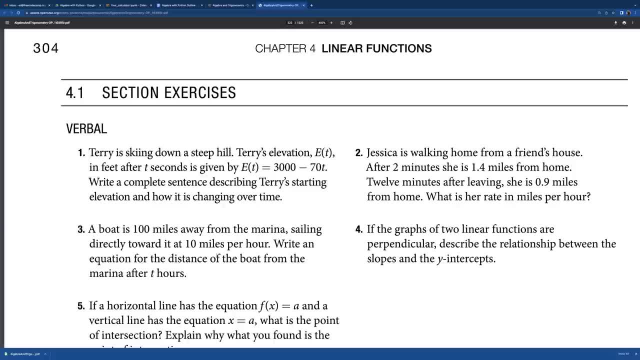 to to get to the marina. um, they're at 10 miles an hour. You might even be able to do this in your head: that it's 10, you know 10 hours to get there, And that's the thing. 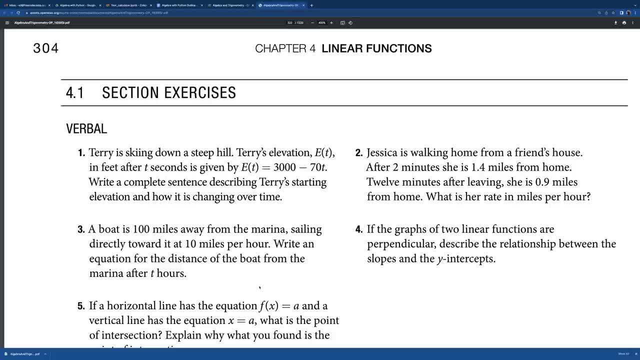 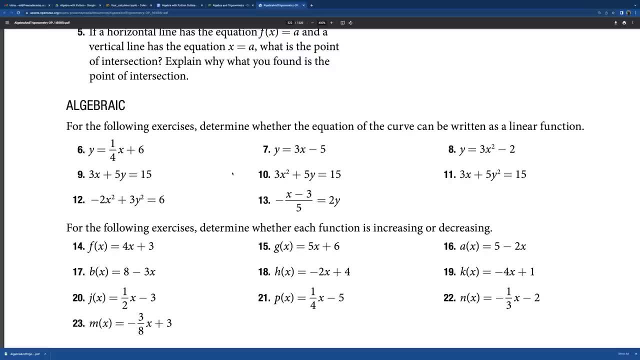 We have the setup for when the numbers get more difficult, but sometimes you can just calculate it yourself, All right, And we take a look at some of these, Okay. Okay, So remember a linear function. we'll get into the other functions, quadratics and things. 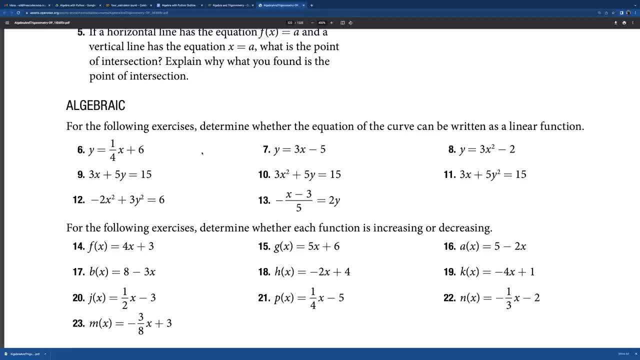 beyond that. but a linear function has no exponents. So there we go: No exponents. So we see, six is linear, Seven is linear, Eight is not because we have X squared. Nine is linear, 10 is not. We have X squared 11.. 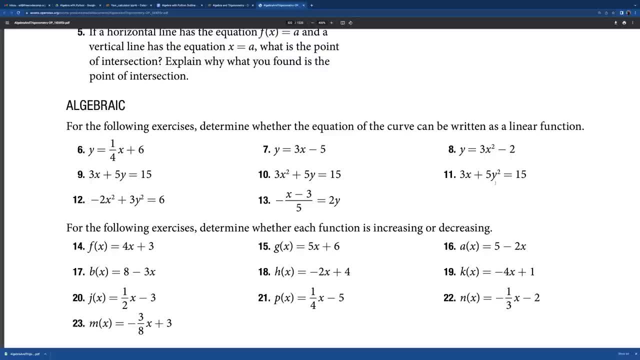 We have Y squared, So that's actually not even a function like the ones we've been doing. So that's another story. 12. Yep, Actually not a function like the ones we've been doing, and certainly not linear. Um 13,, if I had X in the denominator, then that would not be linear, but with just a. 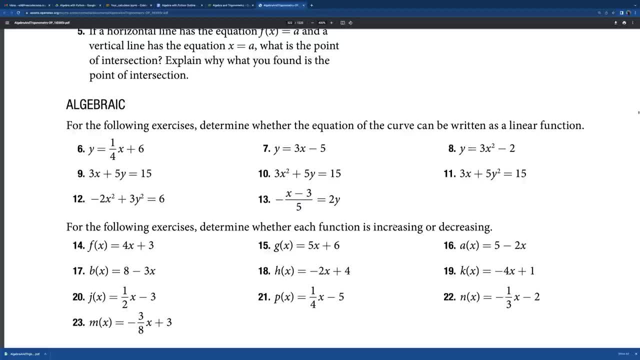 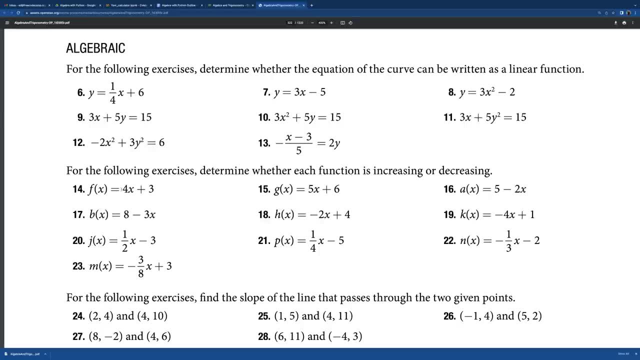 five in the denominator. we're okay. So there we go. And increasing or decreasing, we would just look at the slope. If the slope is positive, it's increasing, If the slope is negative, it's decreasing. And remember, the slope is that X coefficient. 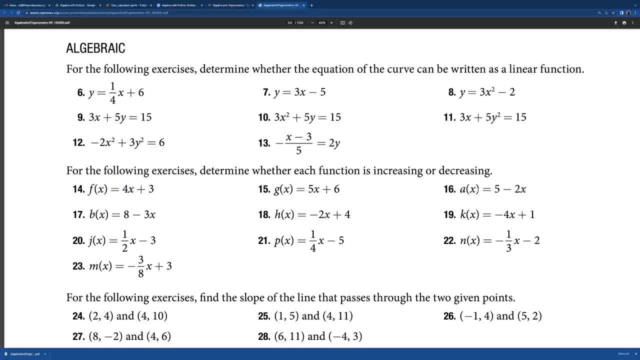 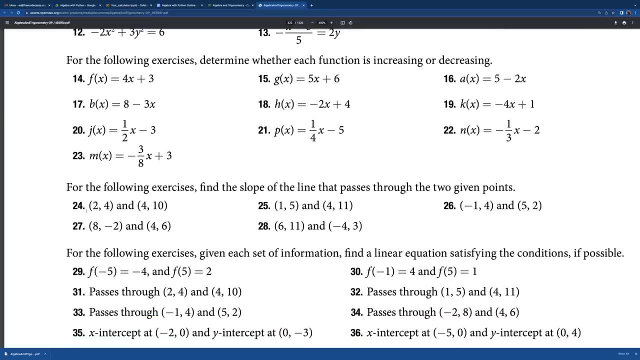 So slopes, for it's increasing. 15 slope is five, It's decreased, It's increasing. And 16 slope is negative. two, So it's decreasing. 17 is negative. three, It's decreasing. So we see that. And just like we were doing with these other problems, you just like number 24.. 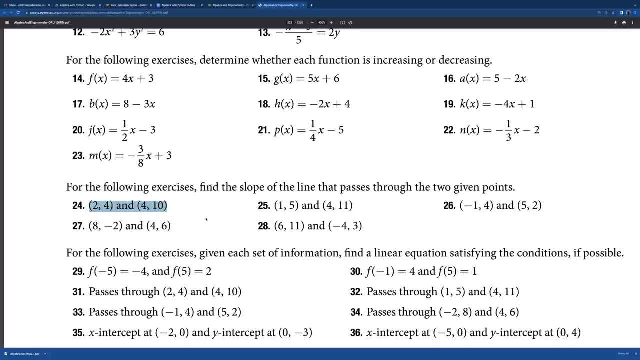 There you go. You could just plug these in: two, four, four, 10.. There you go, Run it And have your equation and see the graph. So a lot of these, you know when, when. once you have the code down, you know it becomes. 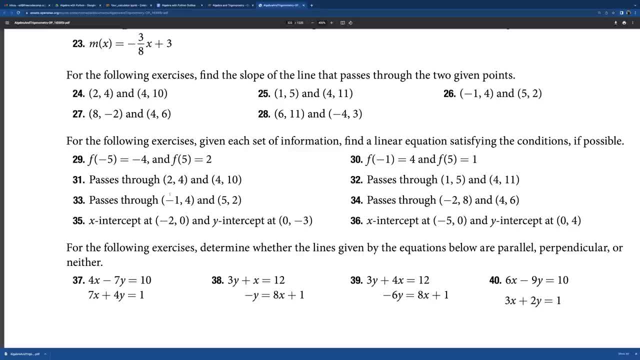 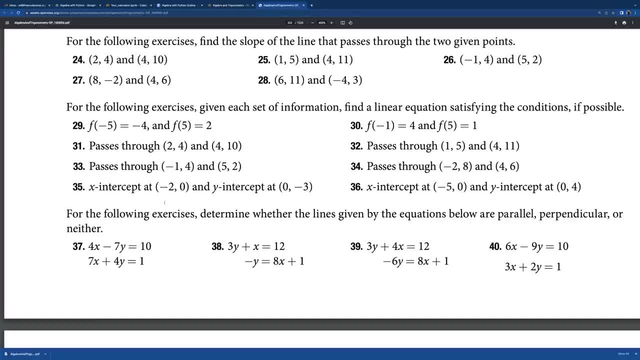 a lot easier. There you go. Same thing, A line. If we have two points, then you know we put this in there. Um, all, right, now let's take a look at 37. So these two lines. now we get into the system of equations. 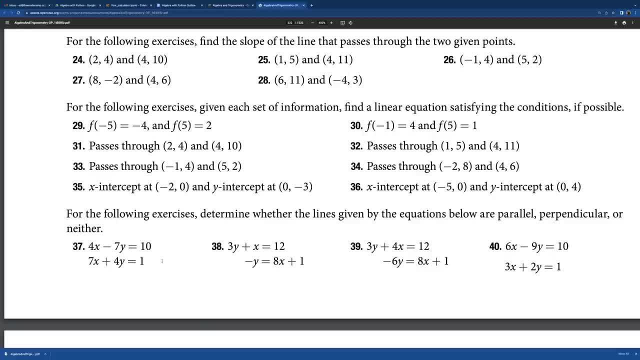 Are they parallel, perpendicular or neither? Well, one of the things we can do, then, is we can look at one of our other uh notebook sections and we can graph these two and see. So let's take a look at this: four X minus seven Y equals 10.. 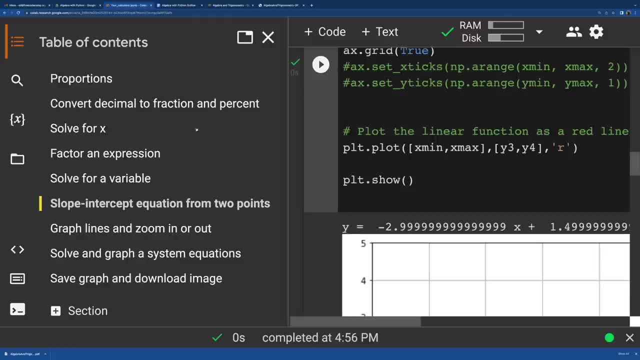 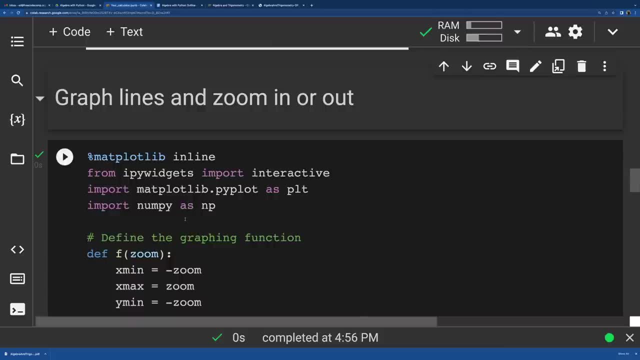 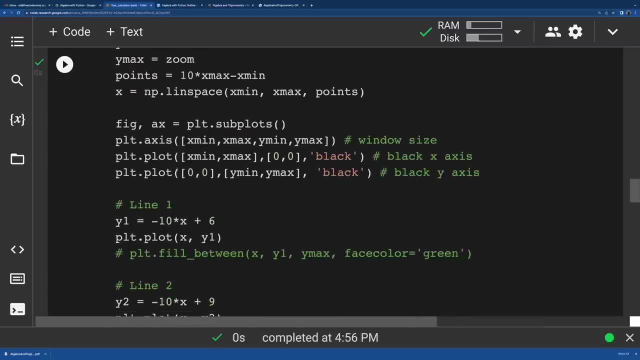 So let's take a look at this, and you would have this- you know how- about this graph lines and zoom in or out? remember? you would have made something like that too, And we defined our function so that we can zoom in or out and we have two lines. 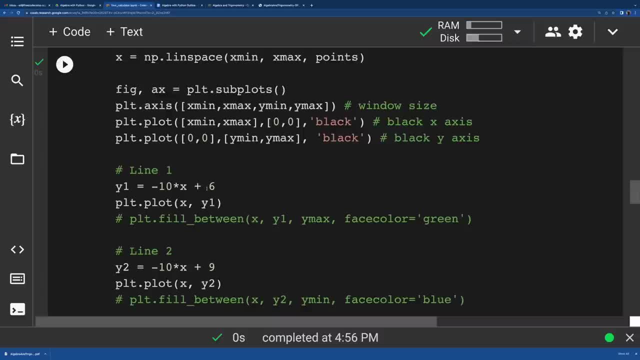 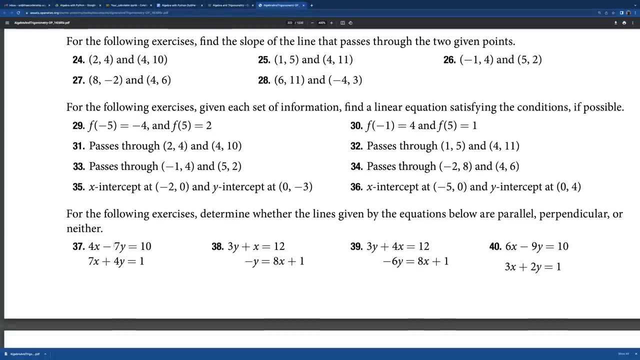 So line one: I could just graph this now also. So one of the things we can do to graph these, if you wanted to, is put it, and this would be something that you would do. You have to put each of these in the Y equals version. 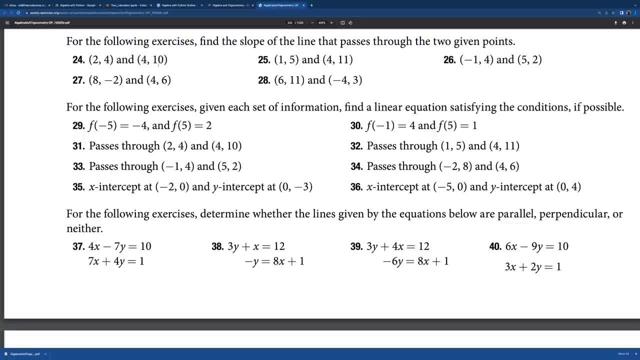 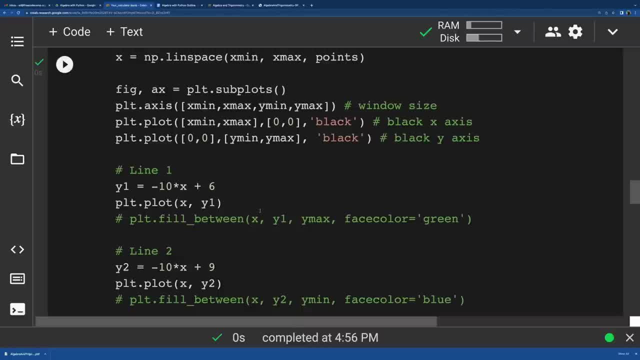 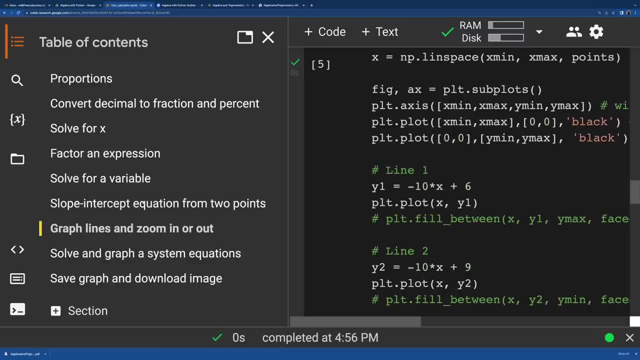 Because, uh, they're not in Y equals and that's how we have it set up to graph. You see, it's it's going to be Y equals and they are going to be functions. So we have this. but let's go to another one: solve and graph a system, because this one 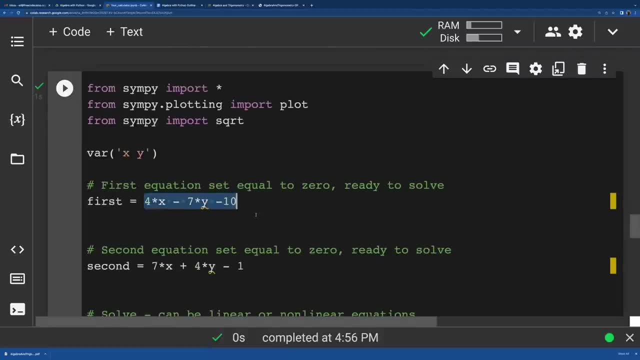 does not have to be equal to Y. In fact, we just make it equal to zero. So I actually have to do this. I actually already put this in here- for four times X minus seven times Y, And the only thing we need to do is make it equal to zero. 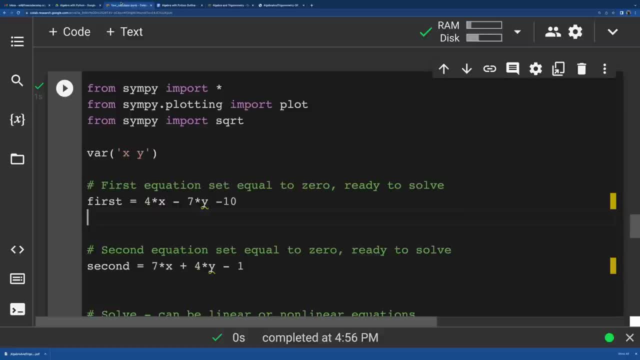 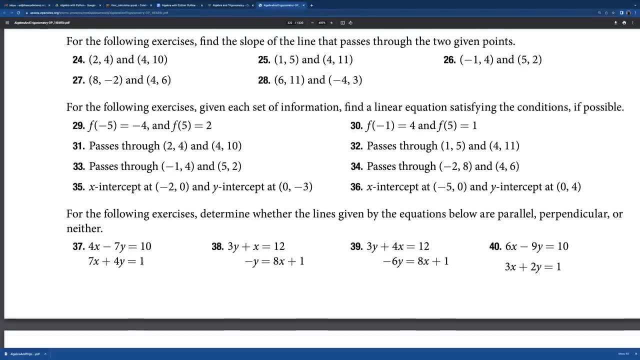 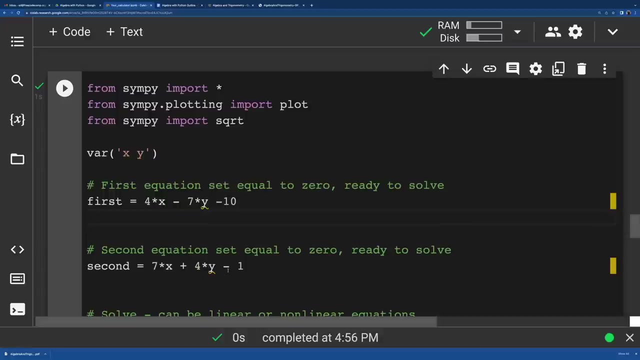 So that equals 10, subtract 10 from both sides. see, much quicker, much easier to do. And then the second one: seven X plus four Y equals one. just subtract one from both sides, And that's what we have here. 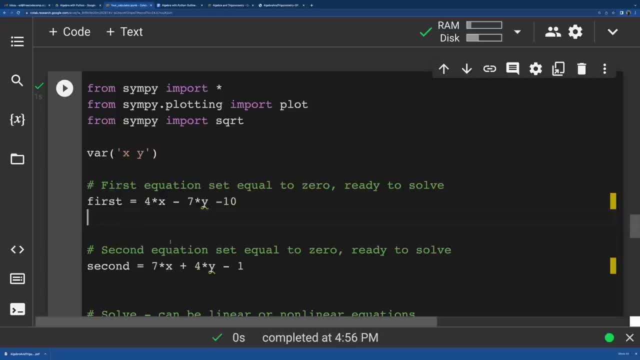 So it underlines these. but once we run it it'll be fine. So that works out really well because as long as you have to set equal to zero just anything on the other side, subtract it over And remember you would have already made this, hopefully. 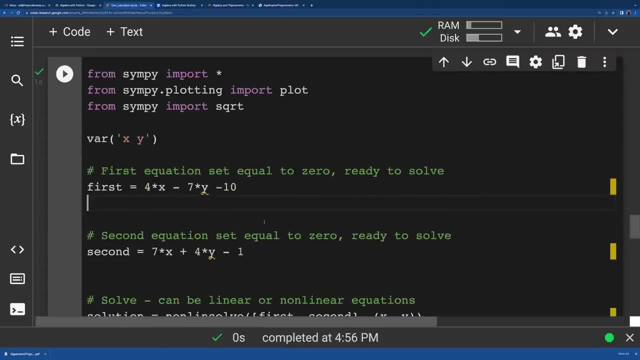 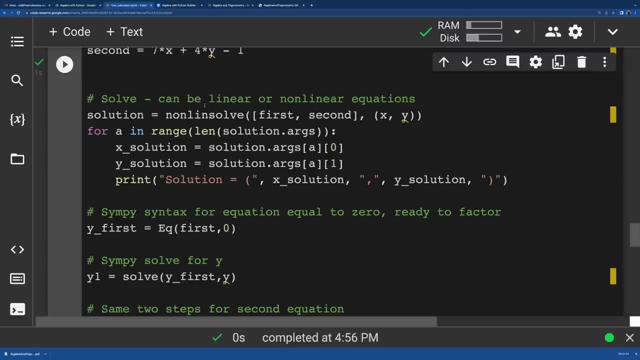 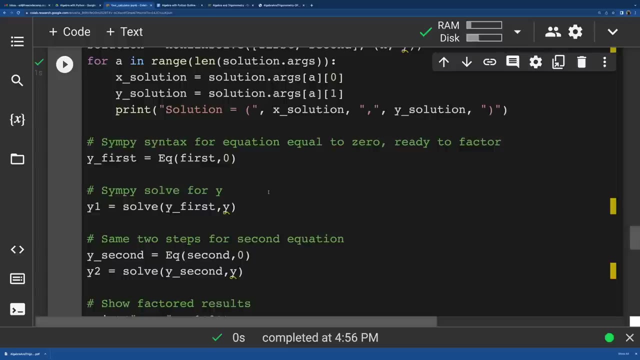 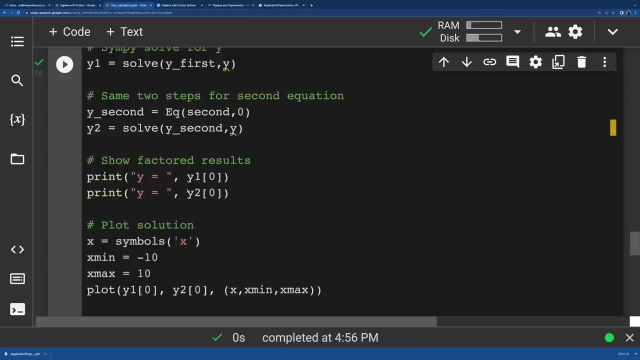 And you know your first equation, your second set equal to zero. And remember, we're solve, then we solve it and we're going to get that solution And then we're going to also convert it to Y. So we're going to print the Y equals here and then graph it. print the Y equals version. 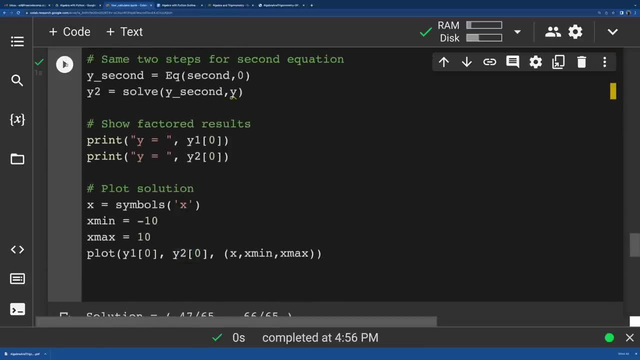 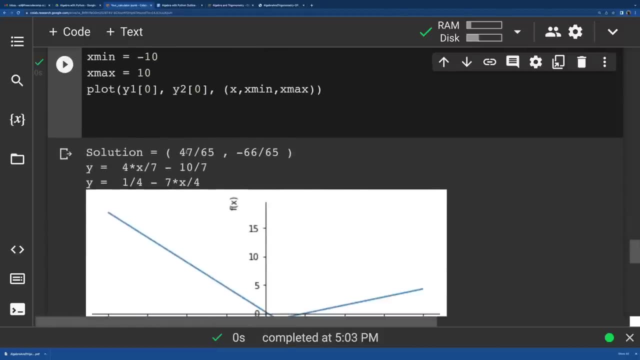 And when we run it, we see we have the solution and it's not even you know. this is again more than the question asked, but if we already had the code, you know we can do this, the solution. And, yes, these are two very weird. 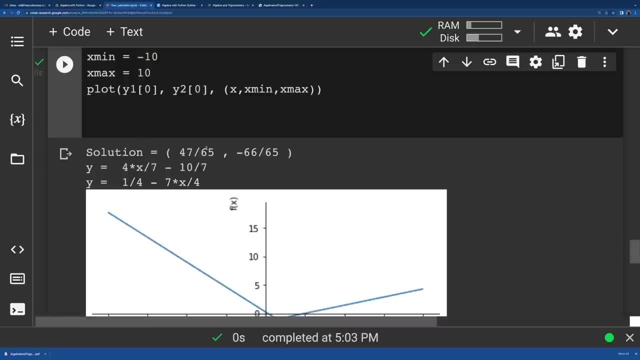 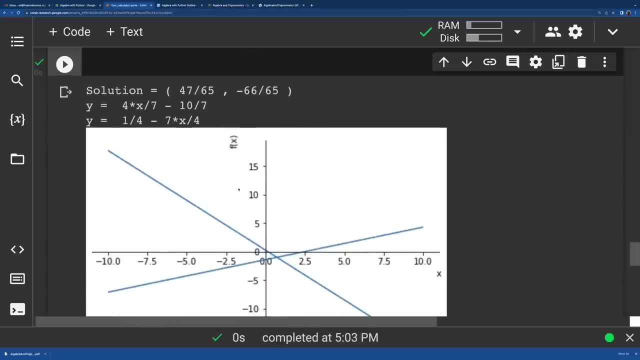 Fractions that you know. it would be a little bit tedious If you were calculating this by hand. we get the solution And so we also see the graph. These are not parallel or perpendicular, and we see where they intersect at this value. 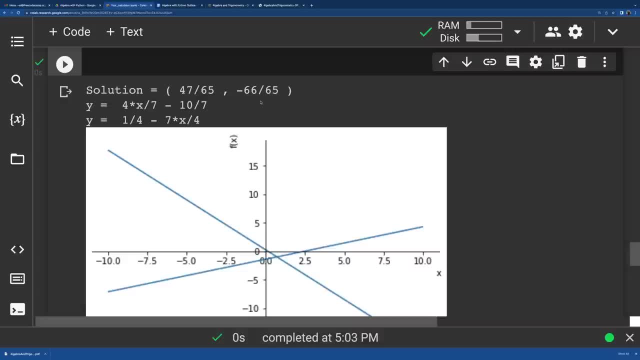 Negative: 66 over 65.. So all you know, almost negative one a little bit off and then a fraction there, And then we see the Y equals versions um four times X over seven minus 10 over seven. So we see this one has a slope of four over seven. 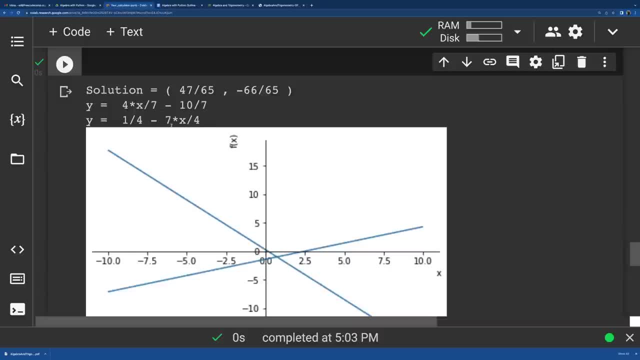 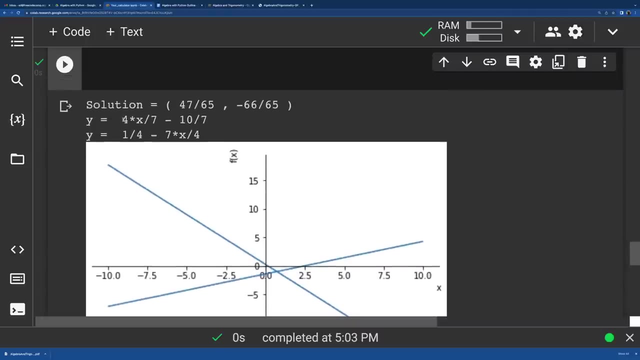 And this one has a slope of negative seven over four. Oh, then they would be perpendicular, despite what this graph shows. So let's try to change this, Okay. So the slope here is four over seven. You see, even though we're multiplying by X, that coefficient is four over seven. 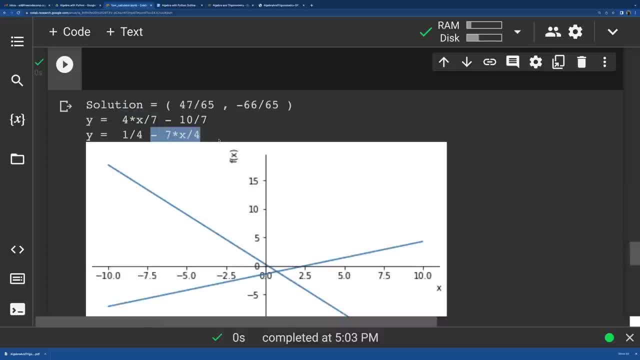 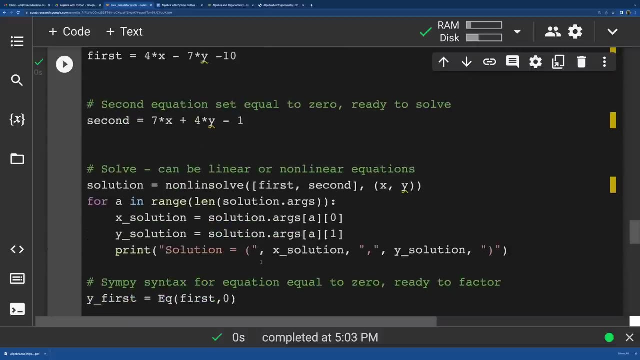 And then over here it's negative seven over four And that's what makes them perpendicular: The negative reciprocal four over seven, negative seven over four, that if you multiply them together that would be negative one. So if we change the scale on this, we can probably, it'll probably- look more perpendicular. 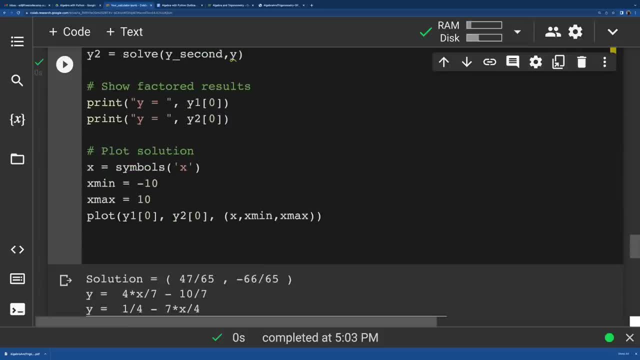 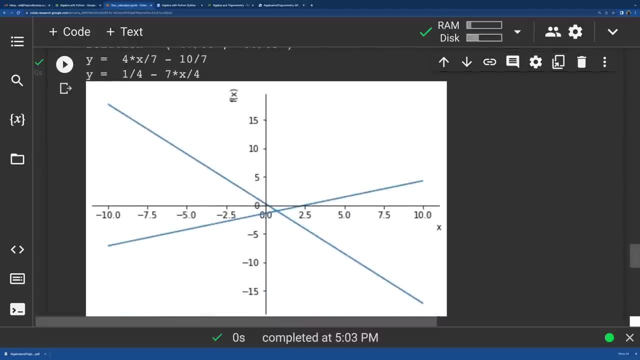 And so this just naturally scales it this way. All right, So we have, but that's why? because in this same window, the Y value goes up to 15. So the you know perpendicular, this intersection would be at a right angle. 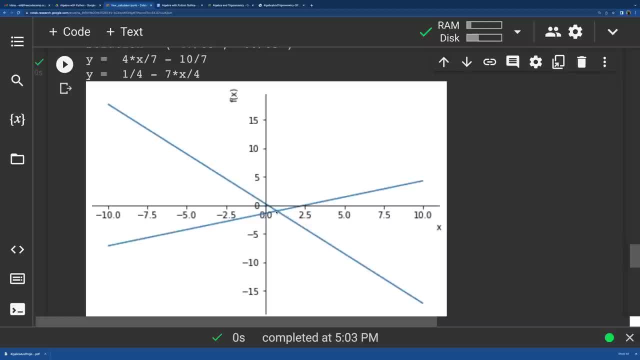 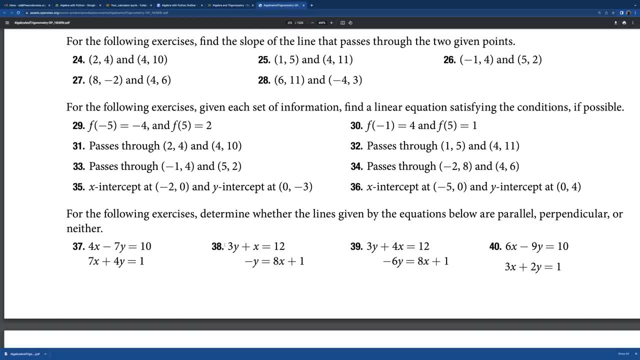 Okay, And then the. you know, we just can't see that right angle because of the scale of the graph. All right, So that work. I would work for any of these. now, you know, 38, yeah, pretty easy. 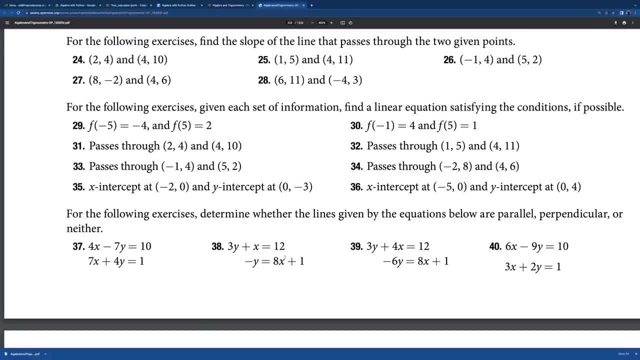 I would just add Y to both sides. you know, subtract 12 on the first one and they're equal, set, equal to zero, And we can use that same thing, Same with 39.. Maybe we'll do. Let's do another one here. 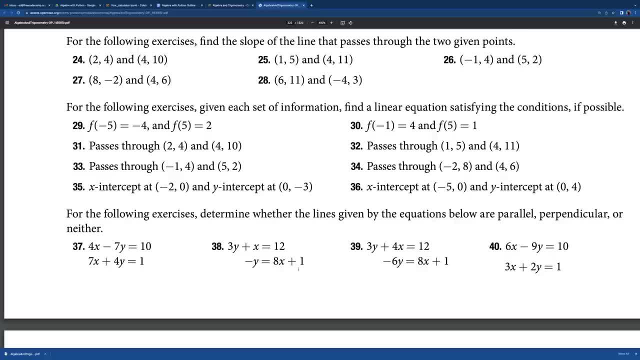 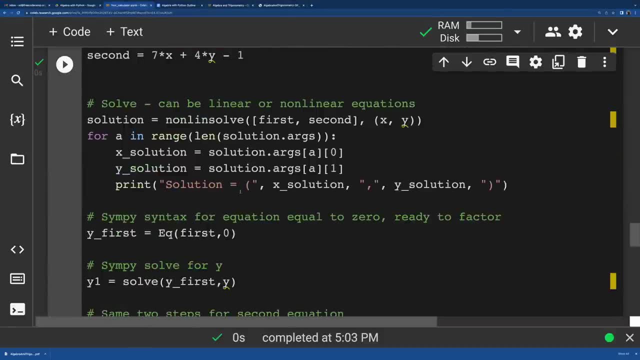 Um, so we get. yeah, if we have this, let's just do yeah, we'll do one more here. Three Y plus X equals 12.. So if we go back to this, then I'll make the first equation. 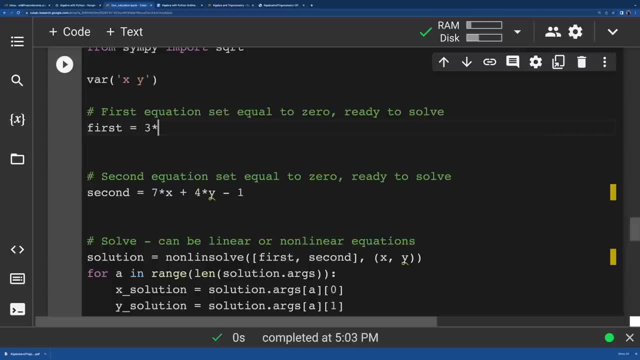 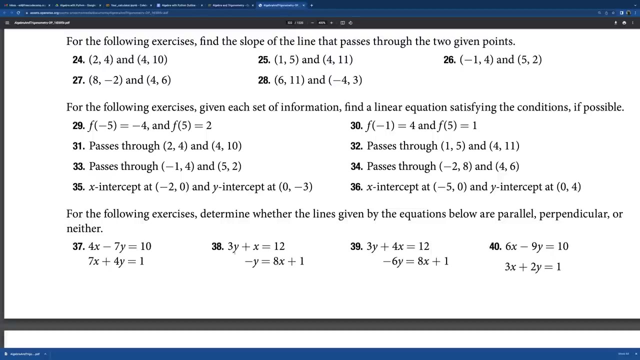 Then we'll have three times Y plus X Minus 12, because that I would have to equal zero three. Remember Python syntax: you have to put the three times Y, whereas algebra you won't see that multiplication symbol in there. 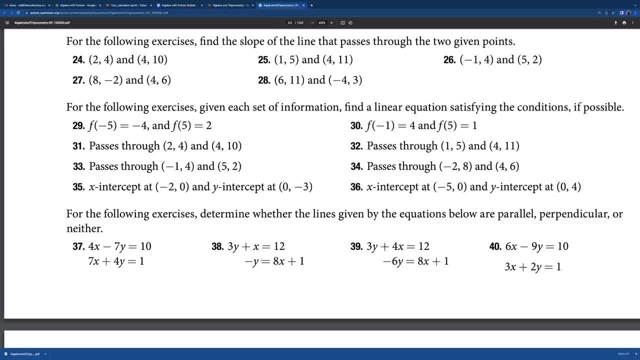 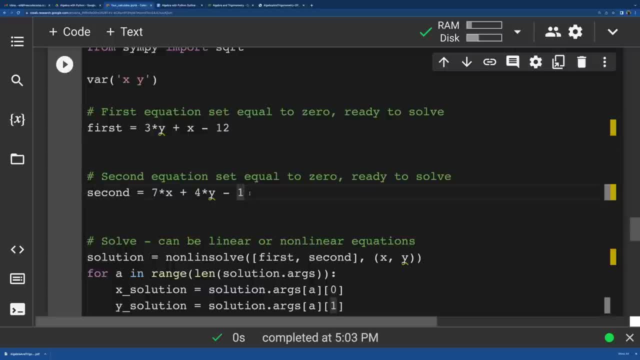 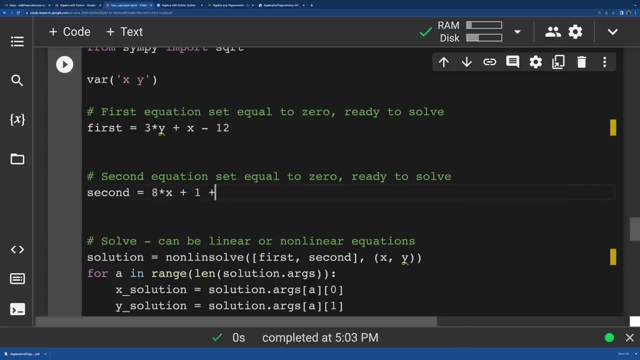 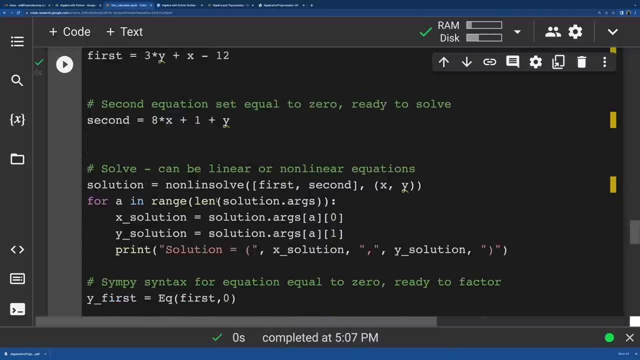 Eight times X plus one plus Y, And see, I don't even these aren't as bad. but you know, for all the ones, you don't have to worry about factoring it, As long as it's set equal to zero. 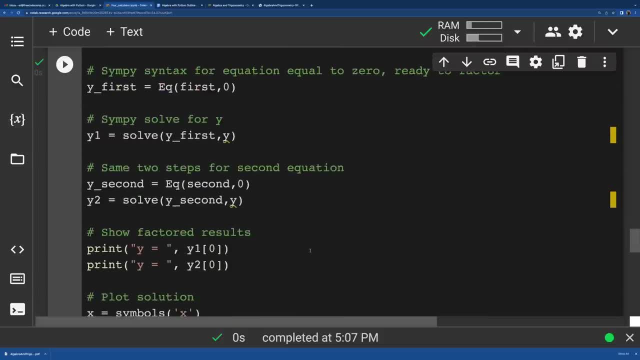 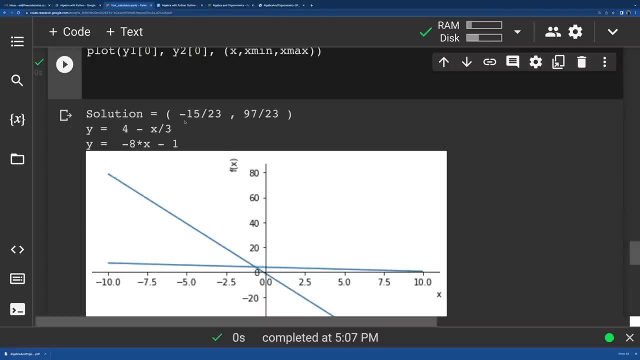 We will get the solution And then we're going to show the Y equals version and then graph it. So, yep, These do have a solution where, a point where they intersect and notice they are not perpendicular because the slope is negative, one-third, you know, 1x over 3. 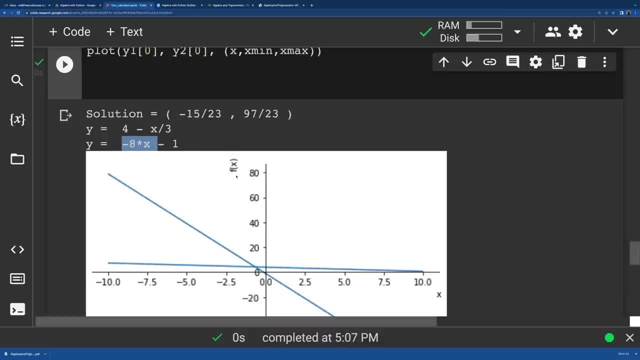 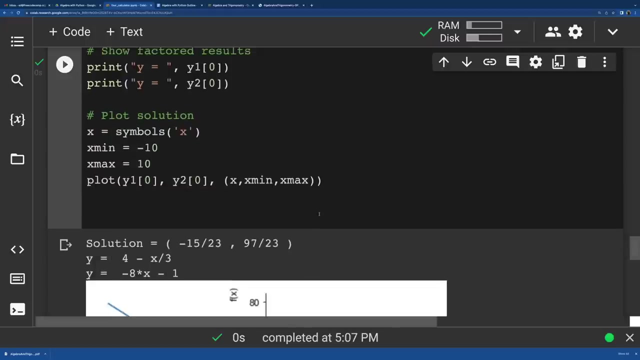 and this one. the slope is negative 8. so a steep slope at negative 8 and also a negative slope, but not as steep. so they will meet at this point. there we go. so pretty cool, solving a more complicated system of equations, solving it, factoring it, graphing it. remember, if you have, you know you build, build these calculators. 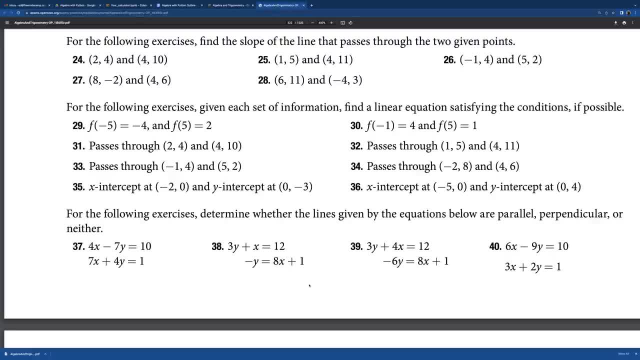 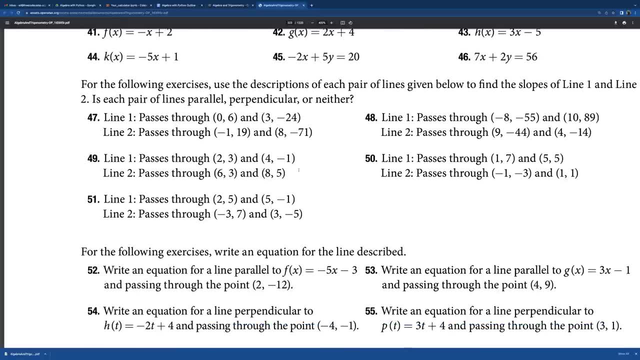 for yourself. then you have it, you can answer all these questions and some other things. and so we see, you know the similar things, lines passing through, and in any of these you could build for yourself, you could build for yourself, and you could build for yourself and you could. 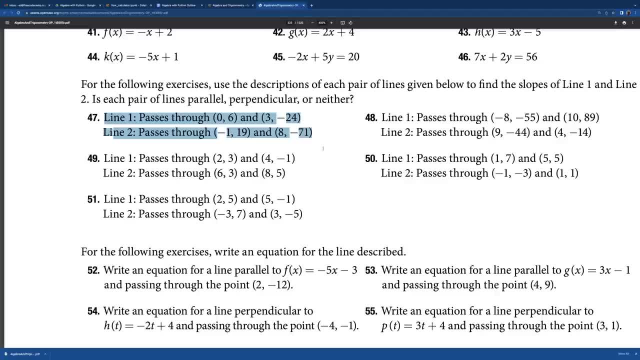 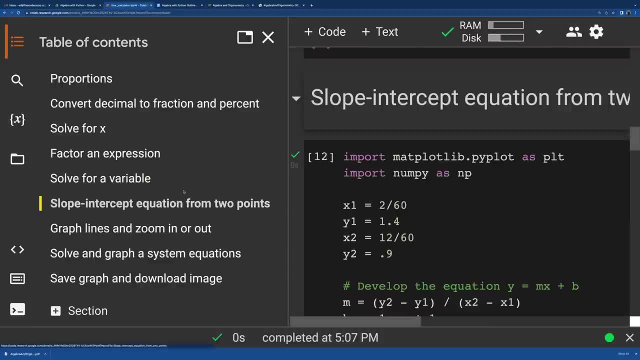 you know a notebook section of code that will do this for two, for two point, two lines, or you could actually go back to the one you had and you could use the slope-intercept equation for the one line and then write it in later, and then you could use the slope-intercept equation again for the second line and 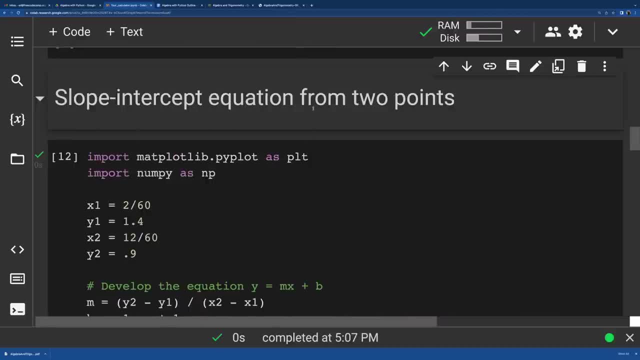 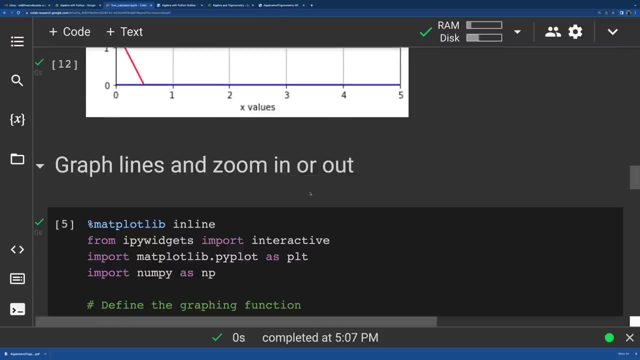 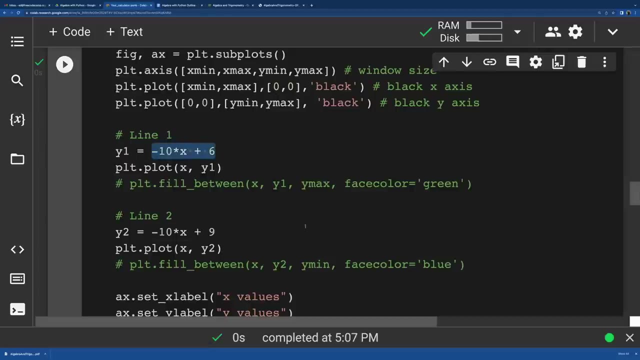 then write it in. so that's what we have here. if there's any skipped from the chart, that if you- unless there is any double career or half career, chilly, brilliant, for you know the like this one- you know you have this slope intercept and you always could then take it and, you know, copy that and write it in here as you. 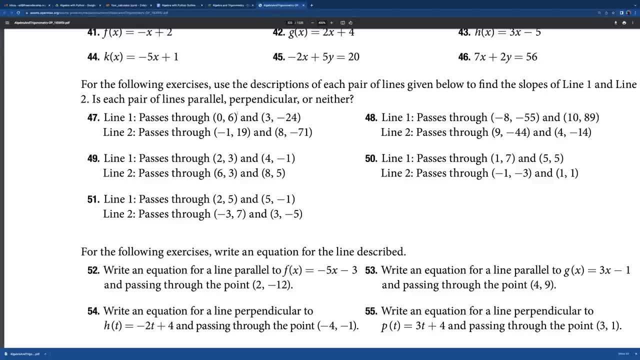 know line one, go back and do the other one, actually do two instead of one, but nonetheless, you know right now, as i have it, it was, it was two separate things. you can get the equation and you could, if you wanted, to copy it into the next one. so all these yep same thing, two points, um, you get the equation. two points, get the equation. 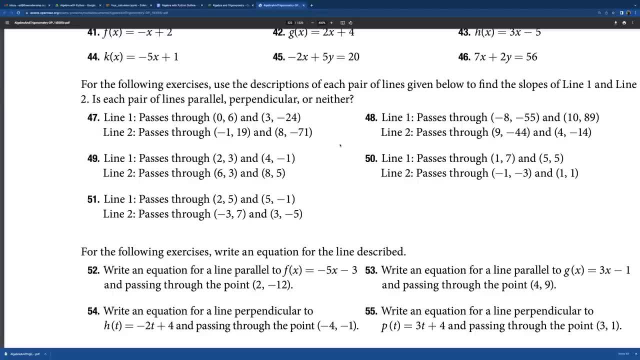 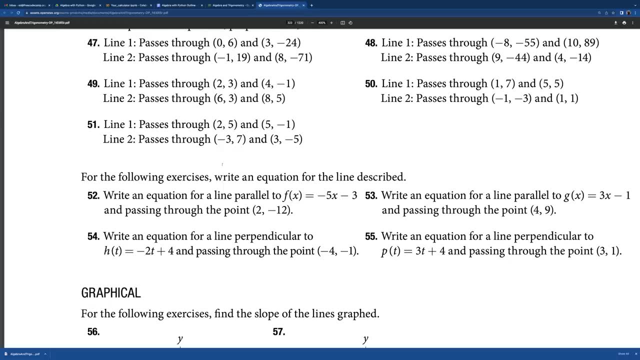 and there we go, just looking at that equation. you know, parallel they'd have the same slope, perpendicular. then you could multiply the slopes together to get negative one, and neither is anything else, as long as they have different slopes. so we see, all these different things you can calculate, and i'll leave this to you, if you. 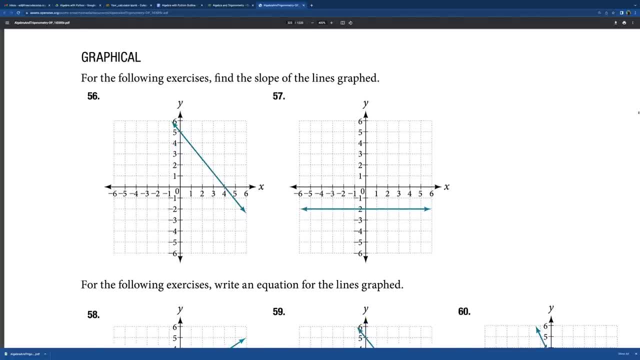 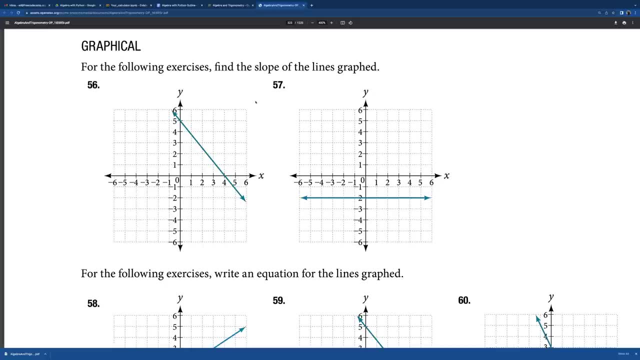 want to, you know, go through and practice some of these. um see, some of these. you don't have to have the full equation or you don't have to have the note jupiter notebook or codemodule have, because if you remember the pattern, that slope, intercept equation here, what's the y? 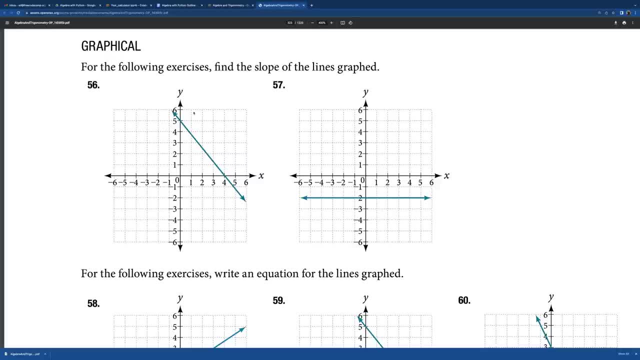 intercept, it's five, you can see it and then, for this particular one, you can actually count. you know, oh, wow, look at that. you know we go down five over four, so the slope would be negative five over four. so it would be: y equals negative five over four, x plus five, or, if you wanted to, you. 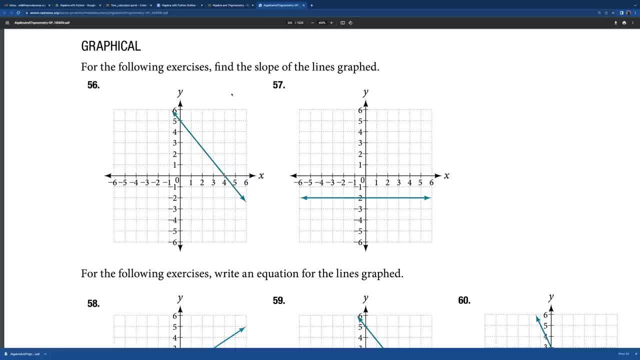 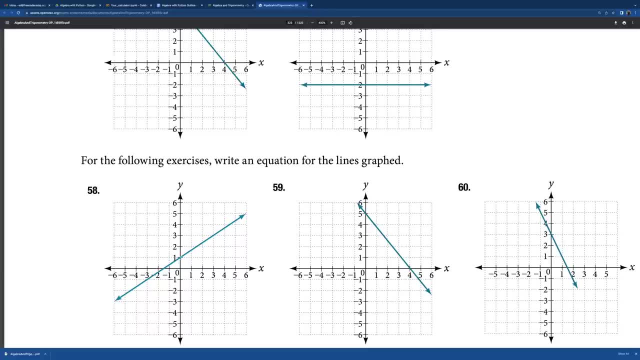 could just take these two points and plug, you know, go back to the notebook, plug them in and see it generate the equation. but see that that'll work for any of these. you know, having this, you can count the slope like in 58. so b is one and then from that to the next nice point, looks like you. 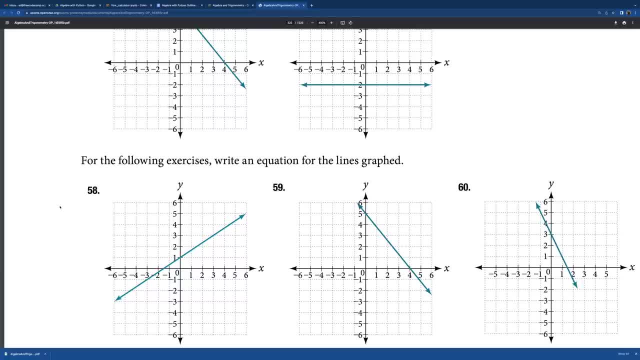 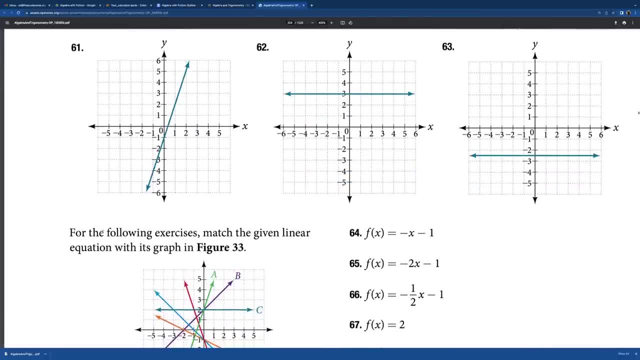 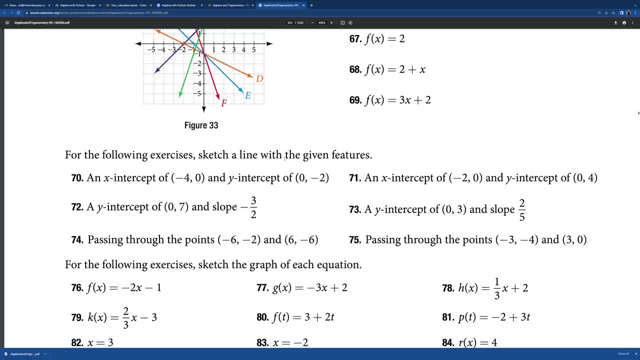 go up two and then over three. there you go, there's your slope, so you can, you know, work on these. so some of these again, any of these. you want to see a graph? uh, you could just plug any of these into that other notebook section where you see the graph. all right, sketch a line. 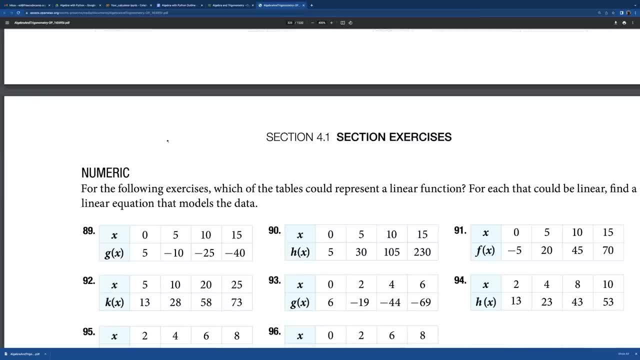 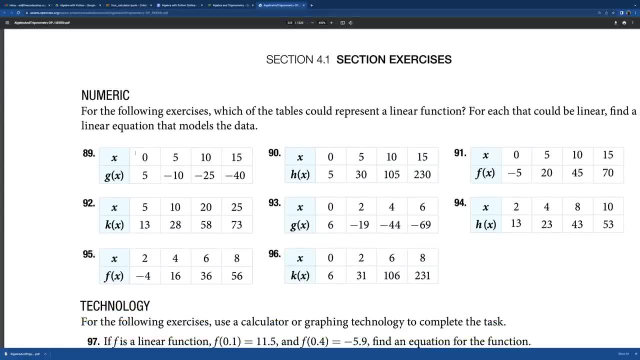 good, and again, you can practice all these if you want the tables. so really just remember x and then whatever you want to call it, g of x, that's the y value, and so you can just plug any of these into that other notebook section where you see the graph. 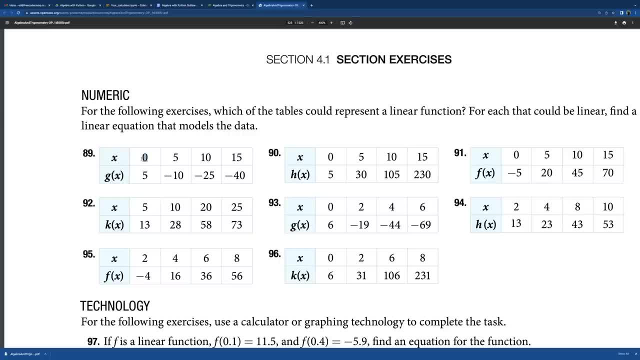 so if i want the equation, then what we want is we can just take the first two points and get the equation. so that's, you know, x is zero, y is five, and the next one, x is five, y is negative ten, and we can get that equation, but then also, if you wanted to, you could get the next one. 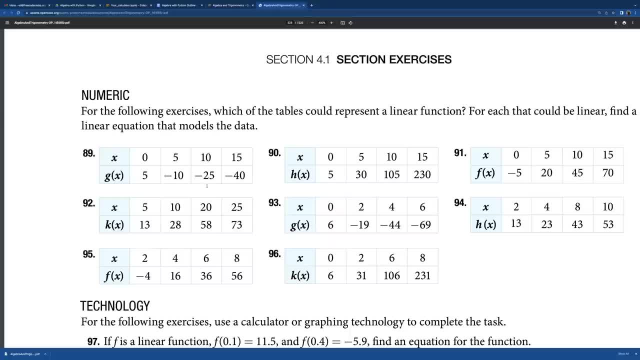 two points and see if it's the same slope. so that's how we would determine if it's linear. i mean, we could always just plot any of these points and and see what it comes out as. so that's another way. we could just plot these points as their own array and see if it looks like they. 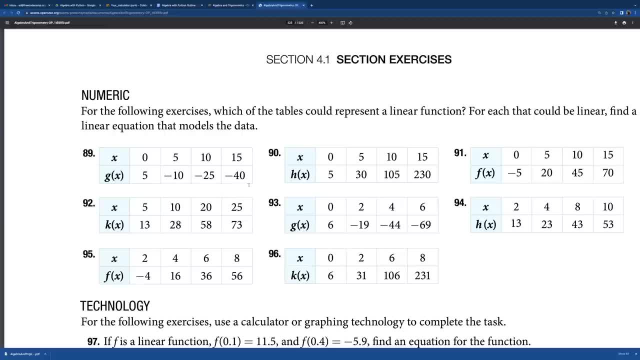 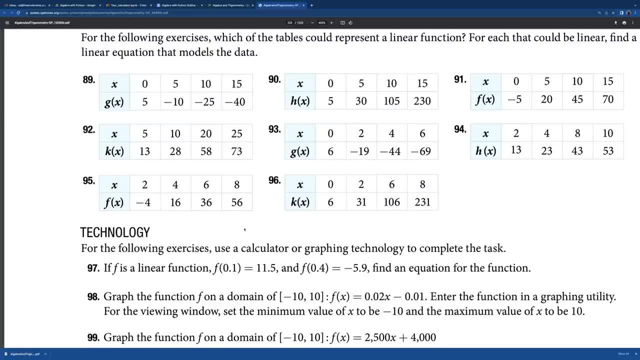 line up. you know, that's another interesting way to do it. and there we go, so, uh, so, yeah, let me. let me just show you how to do that on on one of these. and so if the x value is 0, 5, 10 and 15.. 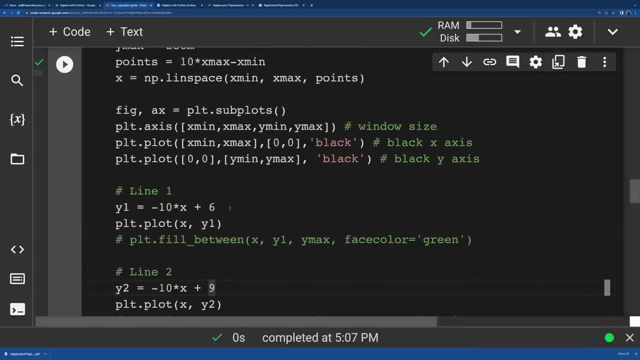 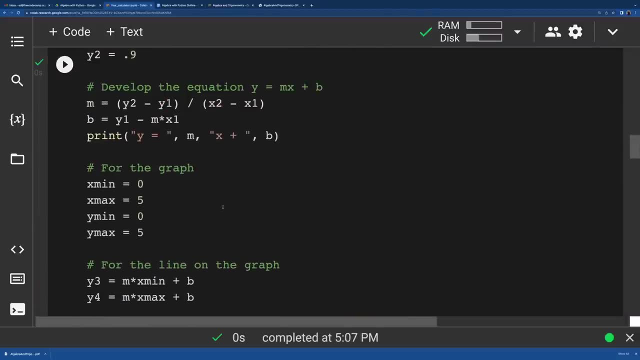 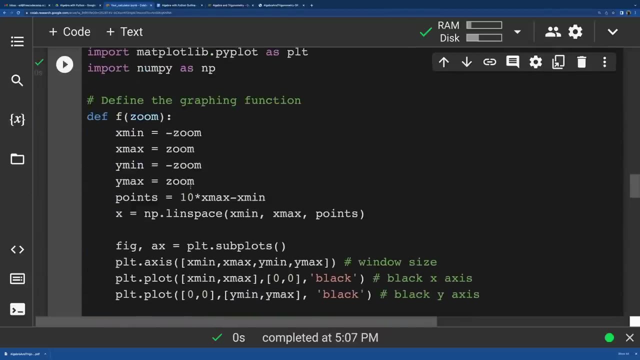 now what you can do is in one of these where you're going to graph. so if we have now here- and we'll even keep the zoom in- so one of these results are gonna be a linear one and then we're gonna put in theчикana. from what we're using, it's gonna be a linear one. so we're gonna put in theчикana and then we're gonna plug into thets like and and a half a step to get to the 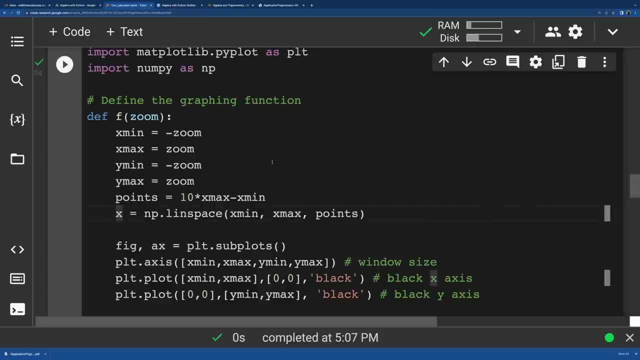 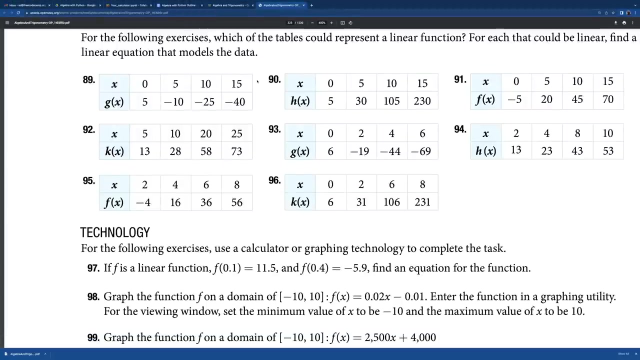 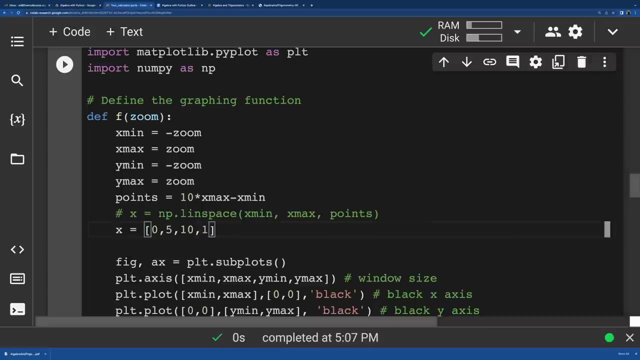 you're going to graph. we have all this for the zoom. but what you can do is you could make an array of the x values Right, so we could get x equals and make it, you know, zero comma, five comma, and you see zero, five, 10, 15.. And we can just make that the array 10, 15.. And then 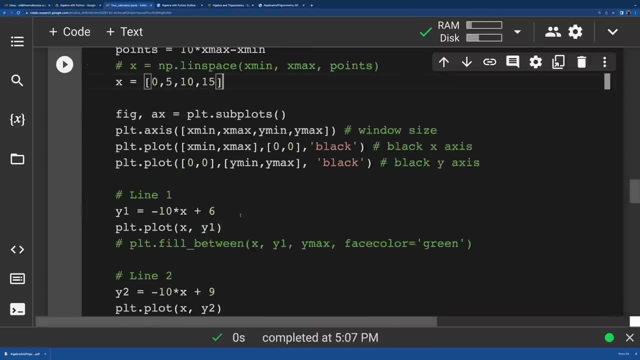 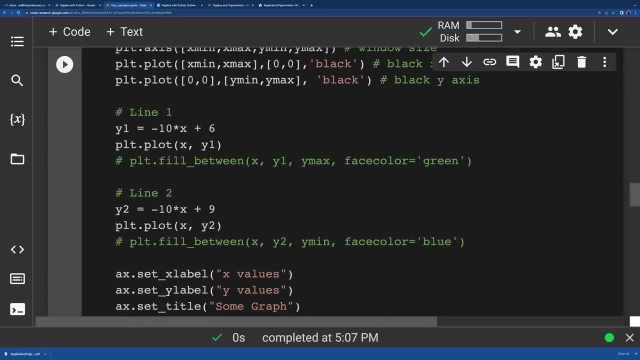 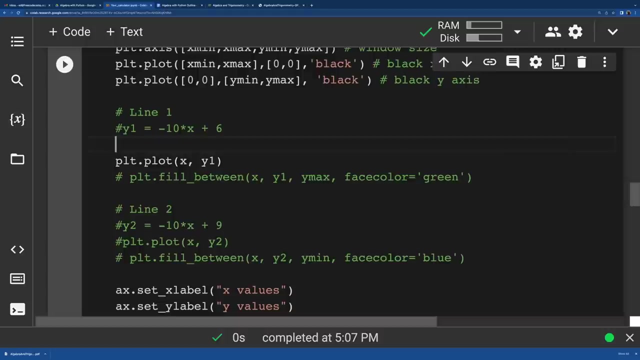 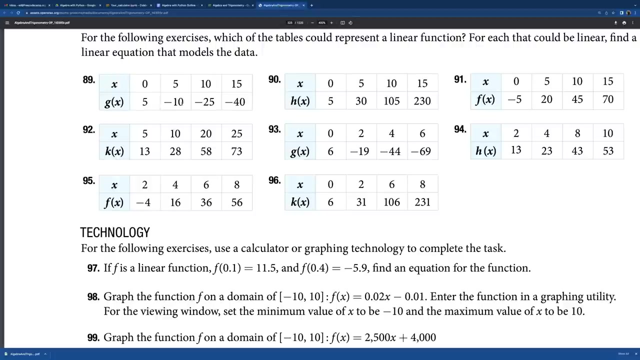 you could now we could just comment out all this, because we don't need these, And take this and this first one we could put: you know, comment out this, And we could have y one and put your y values Five negative 10, negative 25, negative 40.. So there we go. 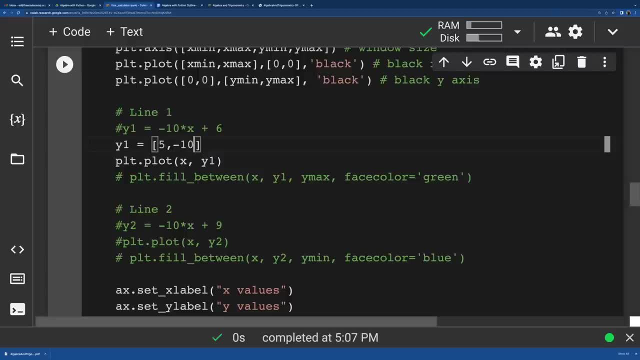 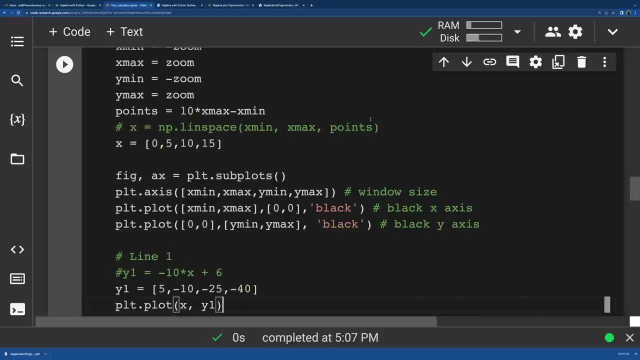 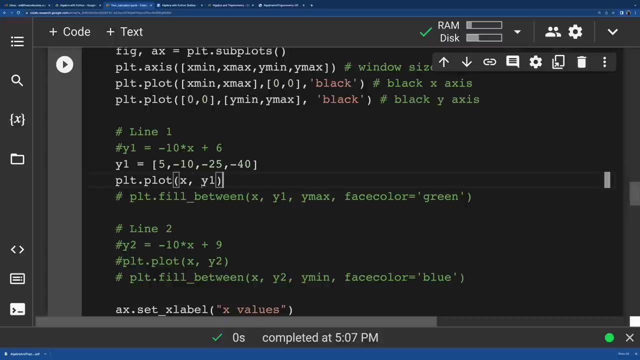 five. negative 10, negative 25, negative 40. So remember that. you know that that numpy essentially does give us an array of values And we could just put our own array And if you wanted to in here, right, we could also then put: 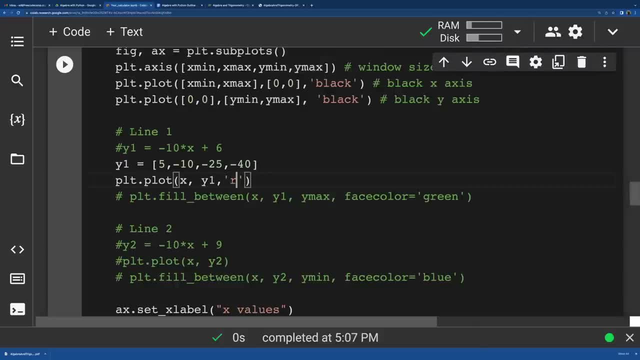 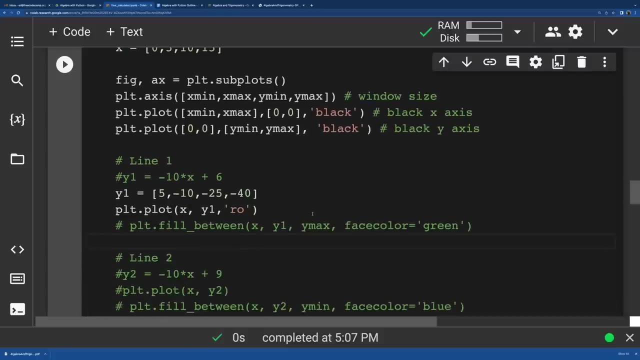 you know, make them, make them dots. I'll say ro, So we'll make them red dots for the points. So we could have the x array, have the y ray, and then that's what we're plotting. There we go, we just 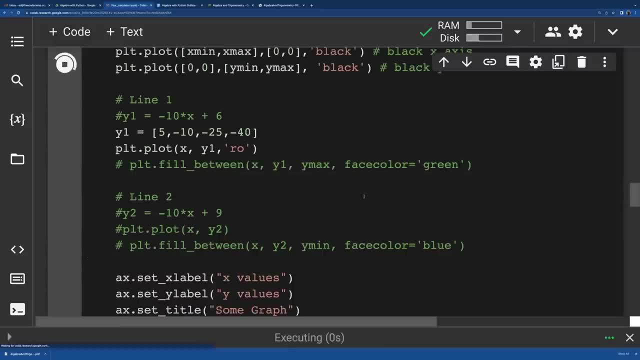 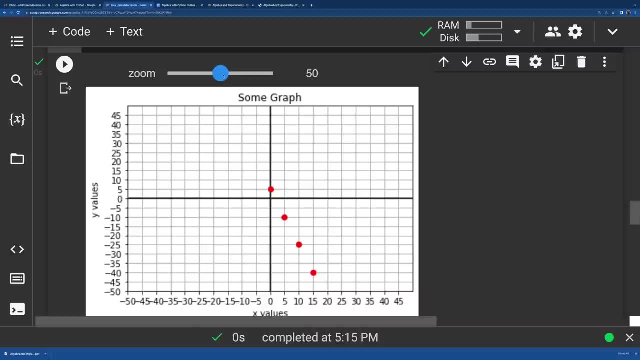 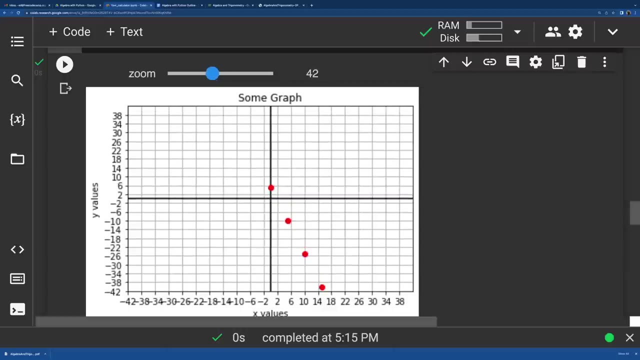 commented all these out, And so we have this looks to be that in line and we can change the scale. I like to keep you know: yep, it definitely looks like they're in a line, So we could, you know, there we go, we could say that, yep, that's, that would be a line, And you know. 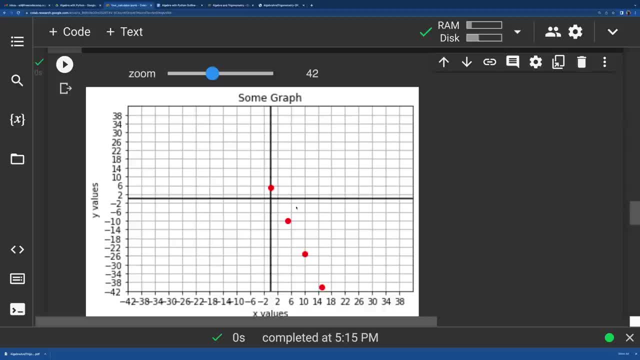 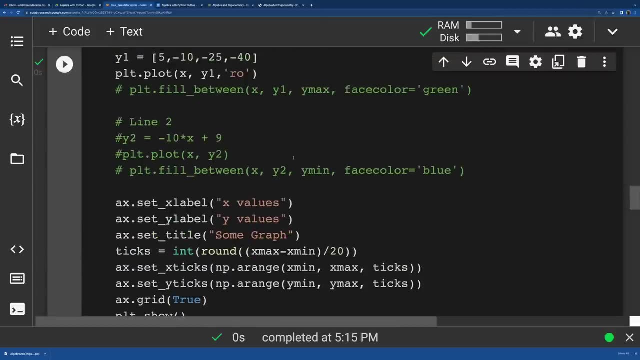 that works. that is linear. So some, some of these you might just notice- okay, does the slope change In in that table? but also i wanted to show you for this or for you know, this might seem like a lot to do for that little question, but also just showing you what you can do if you have, you know. 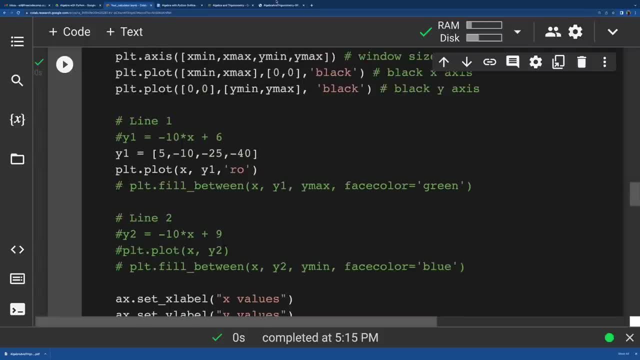 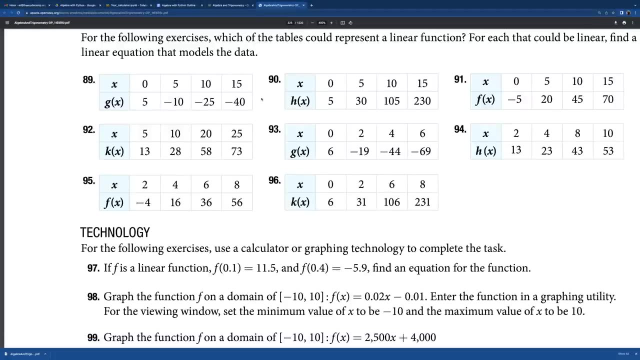 more complicated sets, because all of these that you know, this, this is designed to be practice, and just a few values just to show you. but remember, this is this is going to lead you toward data science. if you want to continue following this path and instead of having like 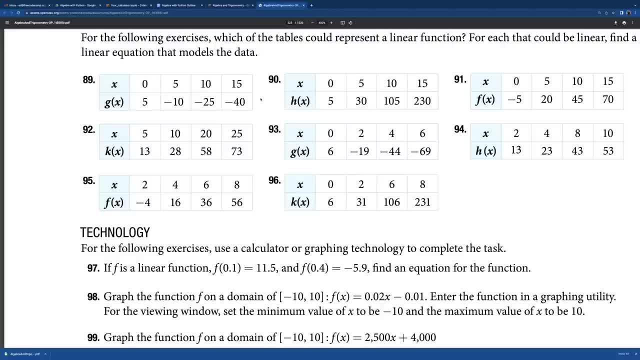 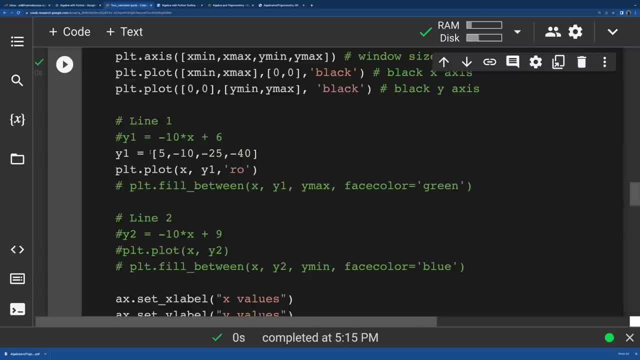 four values you might have, like you know, four thousand, and so we want to know, hey, how can we do this? that we'll have other ways rather than having to, you know, write our own array, rather to grab those values, if there's like a thousand of them, and then store that as an array and same with the 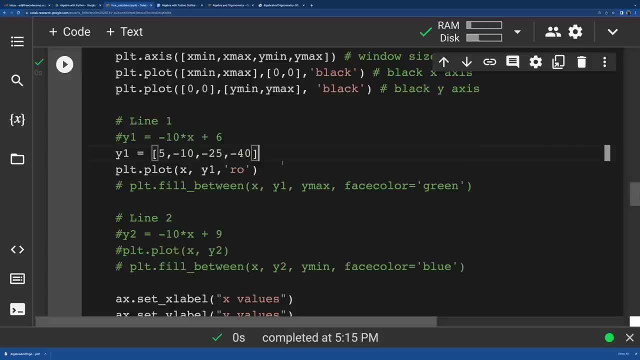 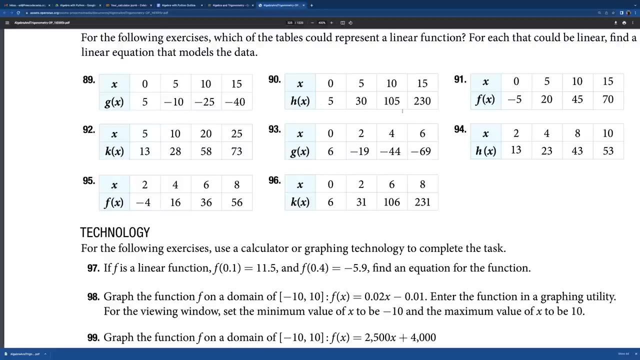 other y values. but then you know, can i do this, can i just take this and plot all these points and see what it looks like? you know, these are the things we want to be able to do. so you know, there we go some, some things you know, and- and it answers a very simple question, is it linear? because otherwise, you know, they might. 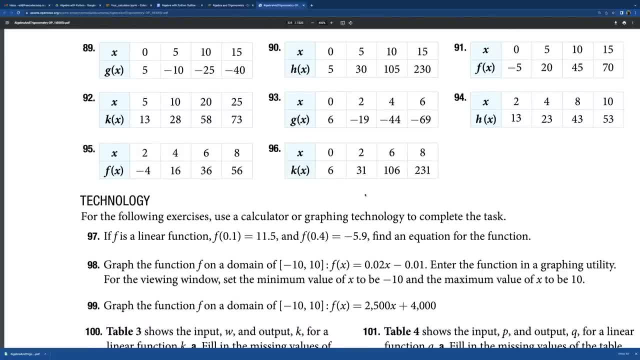 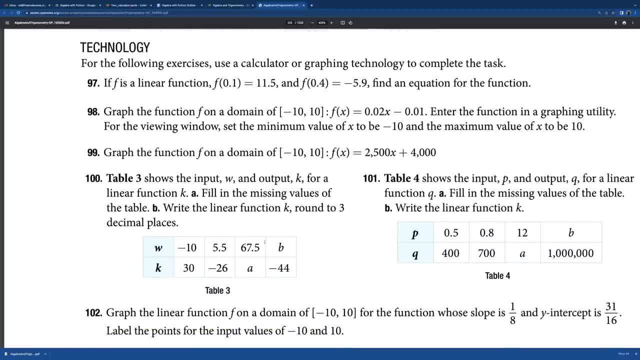 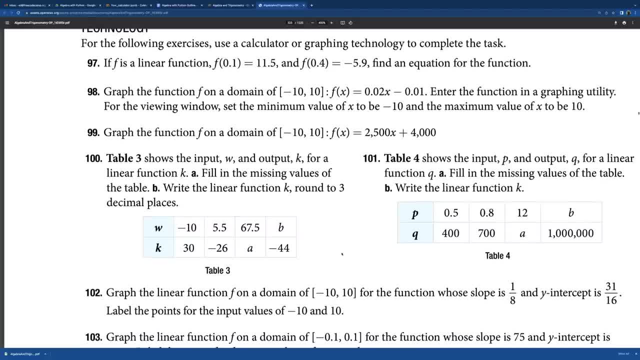 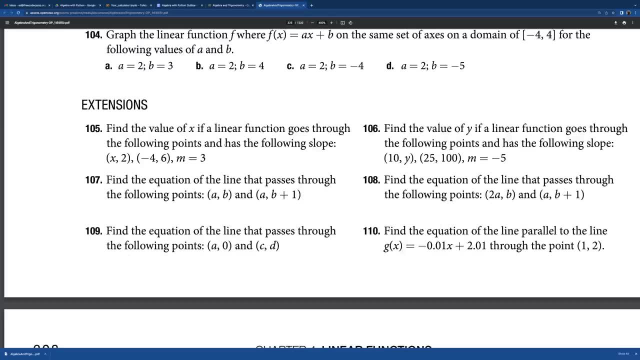 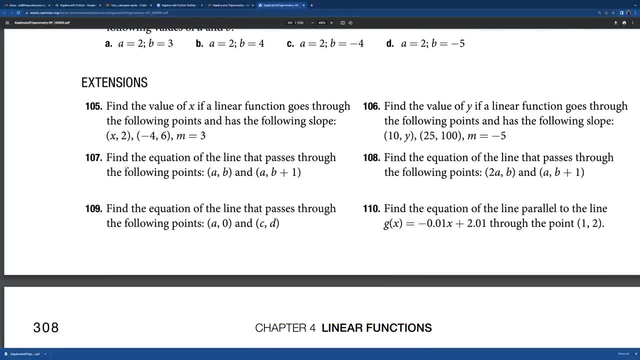 just use some of the thing around. some of these- uh, there are someひ is you can already can introduce a table of values too, if you wanted to. so you know, those are some other things you can do. so we have these and some of these. we would have to put the slope formula. 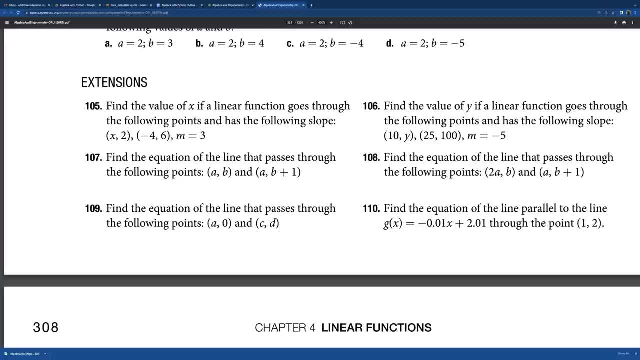 without looking at the code, find the equation of the line goes to the points here. without looking at the code, the y value is b plus 1 and then the other y value is b. so when we subtract that it went up 1, you see the y value went from b to b plus 1. 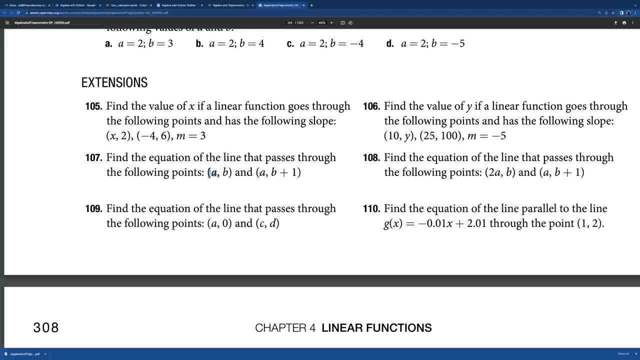 but then look at this: the x value is a and that didn't change. so a minus a is 0. so it's actually not a function, but it would just be an x value. x equals a. so these are some of the things, just plugging in these values. 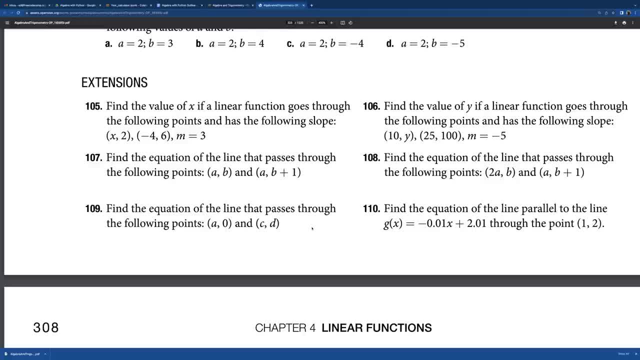 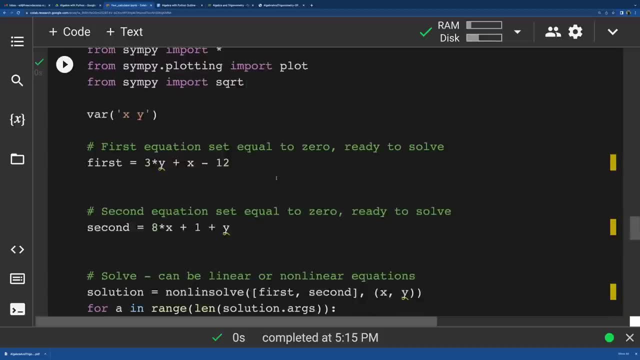 in the slope and you could always do some of this with. you could define all of these values. if you look at the other one that we were doing here- solve and graph- now you might- you might have to comment out the graph. probably wouldn't do too well. 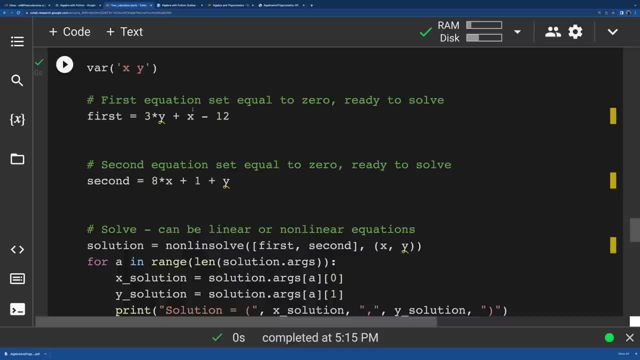 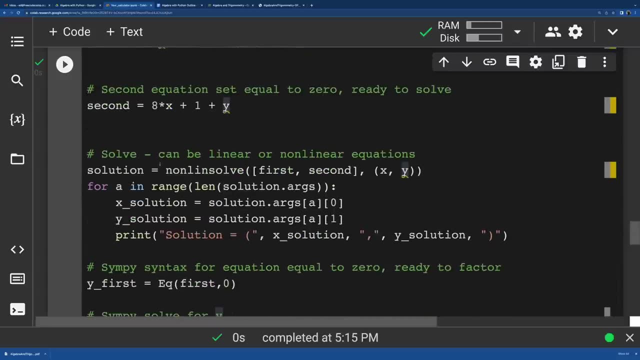 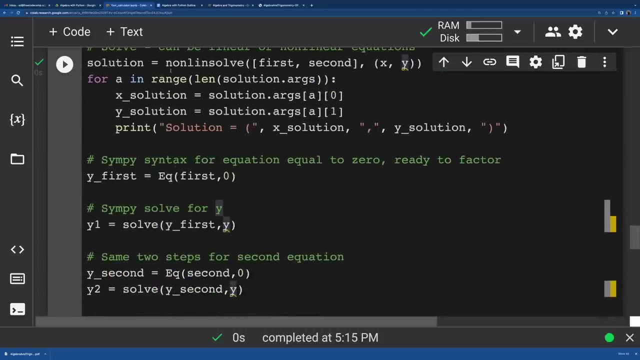 but taking these- and you know, you know, if you define more variables, you could still take these and define these values again. the solution might not be really possible, but you could take those values and then you could actually solve. and this solves it for zero, but you could actually solve it. 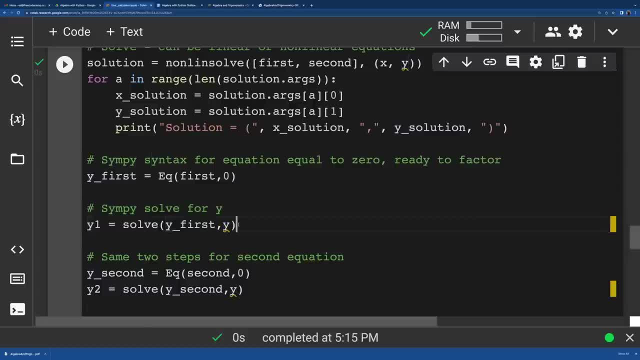 for solve it for y or whatever value you want. so simpy will do that for you. so that's it. you know you could have. you could have a make another section in your notebook that just does all that interesting factoring. all right, so there we go. 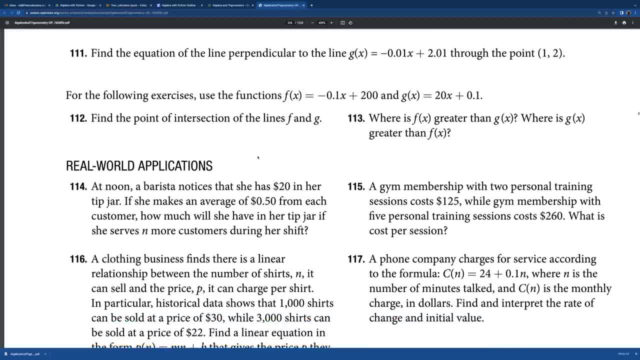 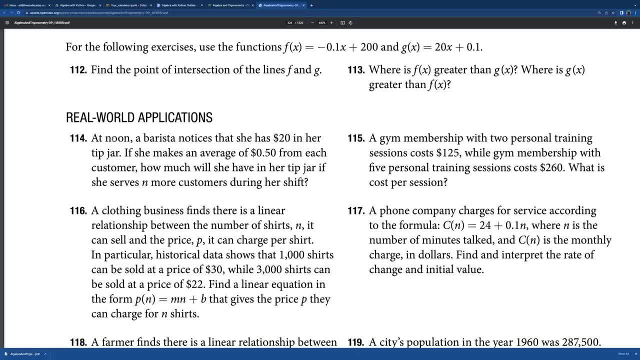 and so we have some other ones here, so so here's one that's a little bit different than the other ones that we were doing earlier. so so here's one that's a little bit different than the other ones that we were doing earlier. so so here's one. 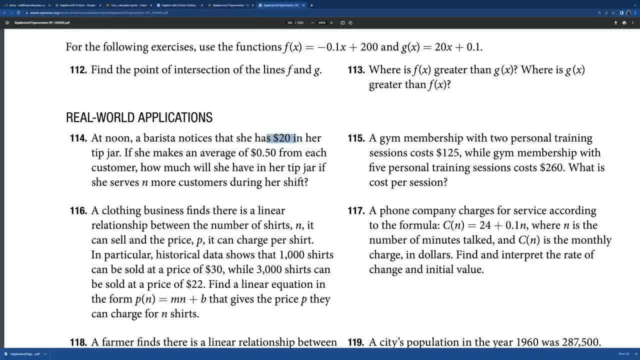 now this. we have noon. the barista knows she has $20 in her tip jar and if she makes an average of 50 cents more from each customer, so remember that's an average. so you might have customers tipping more, some tipping less, and then it averages out. 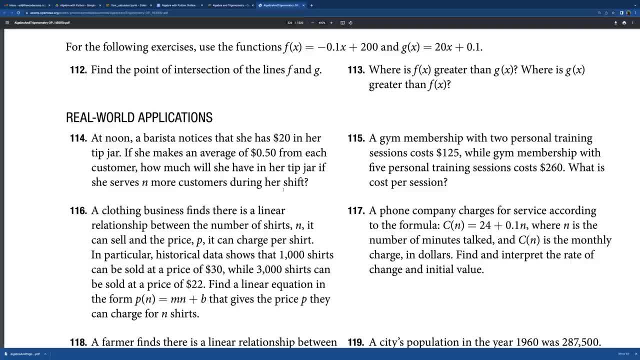 so. so these are good estimates because we we right away see the equation. we begin with 20 and then it's an additional, because you know she's getting something more than the average. her tip jar would be: if she makes an average of 50 cents more from each customer. 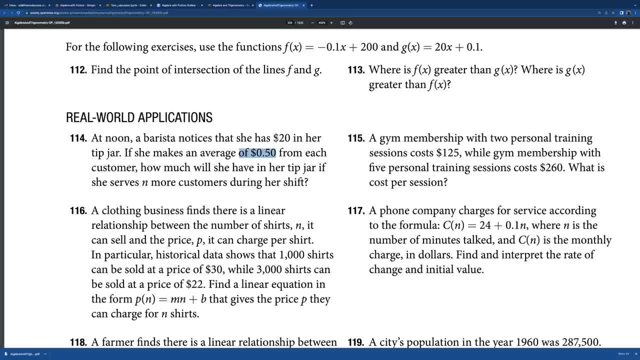 more 50 cents from each customer, so it's 20 plus 0.5 x. so we see that equation. then we, you know right away, we have that 20 plus 0.5 x and we can do something with that. we could like graph it we. 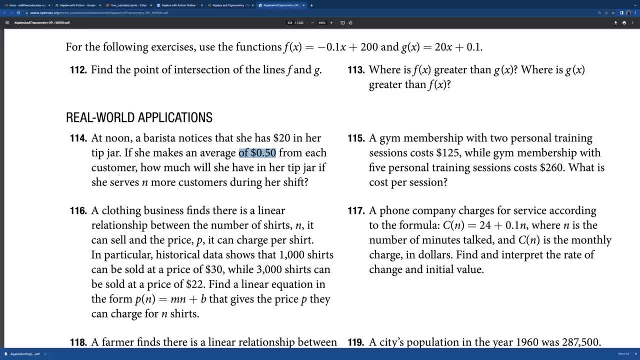 could find values um this particular question. we just says n more, so it would be 20 plus 0.5 n. you know, we just change that variable and then at any point she can plug in a number for n, figure out you know how many tips she has. all right, and there's 115. these are some of the 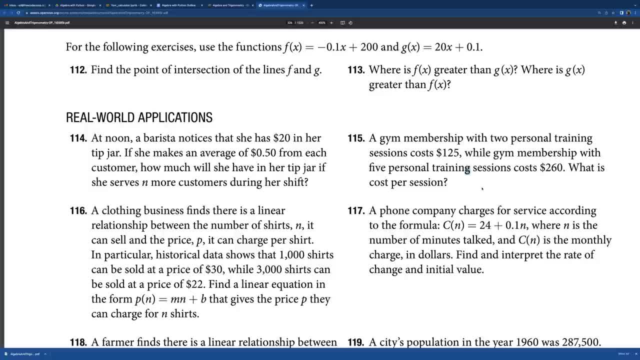 things that you know. you can calculate: a gym membership with two personal training sessions costs 125, while gym membership with five personal training sessions cost 260. what's the cost per session? so we take it as the membership itself is just one thing, and then you could have, like you know. 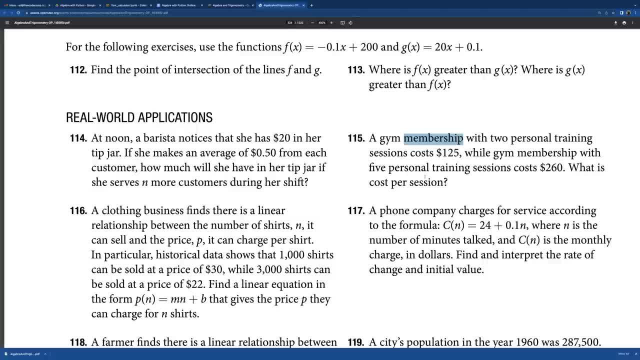 each of these. so really we have our x value would be how many training sessions, and then the y value would be the cost, and so that's it. even though you know we don't- it's not asking us to graph- we absolutely could go back to this and two sessions. 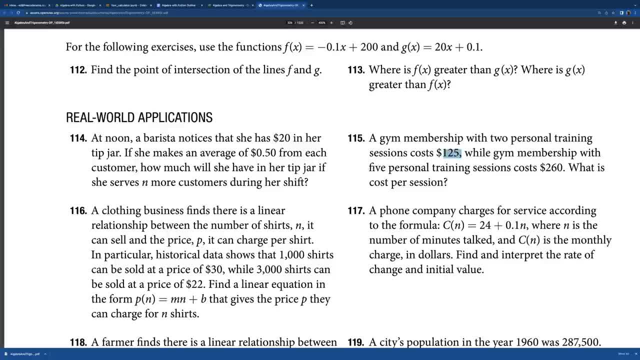 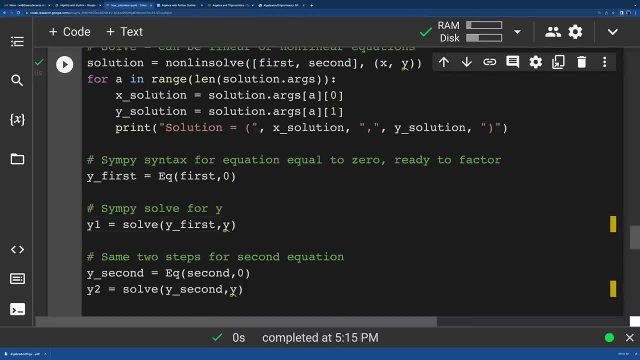 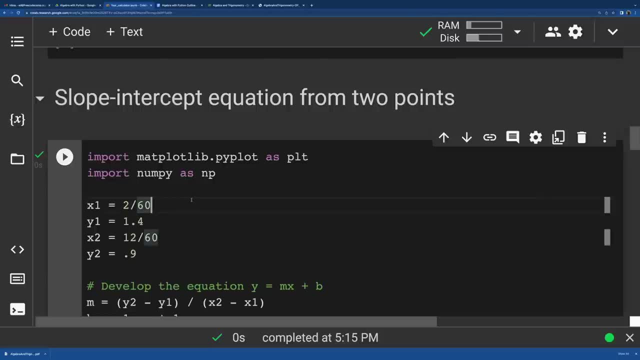 you was 125 and then five sessions was 260. so we could go back to this and back to the earlier one. you know slope intercept from two points and we could say: you know, there we go, two sessions um costs 125, you know how many sessions, and then dollar amount, and then we have five sessions. 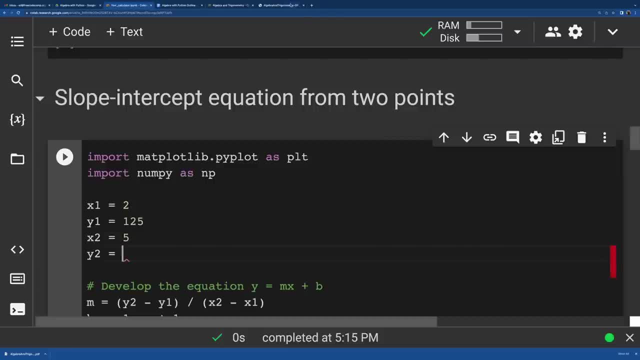 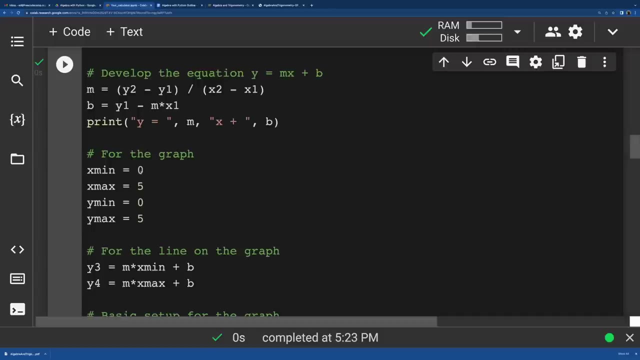 so sky large. bueno, do in lego would be than too sixty and oops. ah, now this: we need to change this. that X minimum. now that's probably fine for five, but let's take a look at this and you'll have I don't know. let's go up to ten why minimum two is still gonna work. b hotjaws would be okay. so then I think that was a match. by the way, 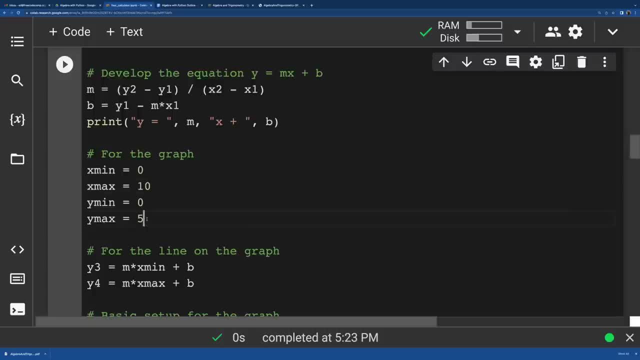 don't we have any question about this stuff right now? oh, it's gonna be no fucking panic, no questions about this, All about the events. and all this stuff right now IS NOT the same question. Minimum zero is probably fine, but the Y maximum, and there we go. 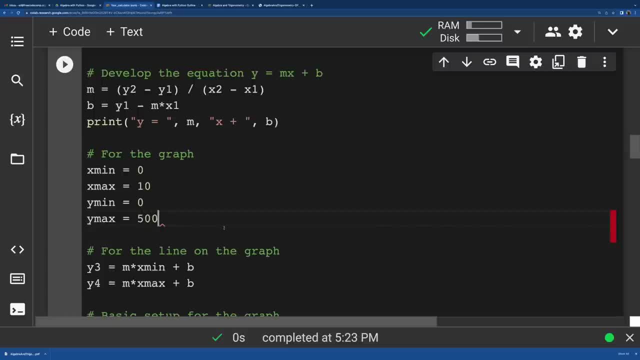 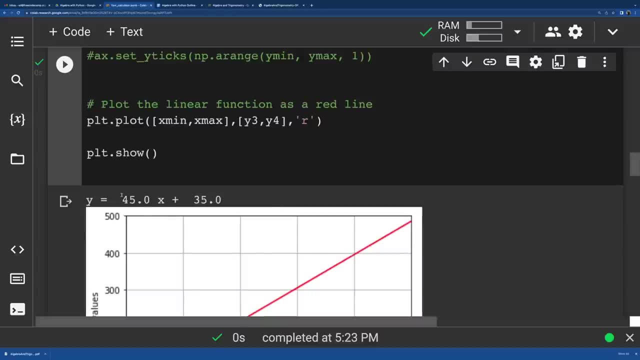 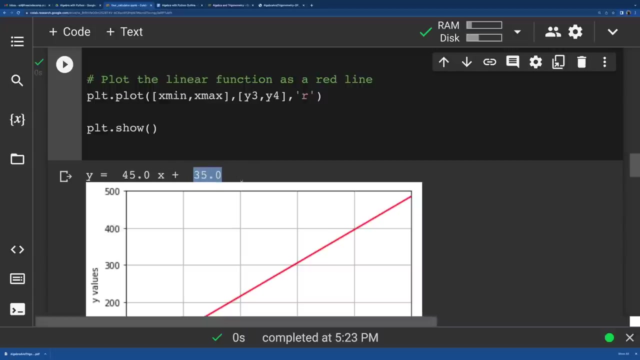 Maybe we'll make it, like you know, 500.. We're going to go beyond that, but that's fine. And we see the graph. So we see the equation: 45X plus 35.. So the membership itself must be $35.. 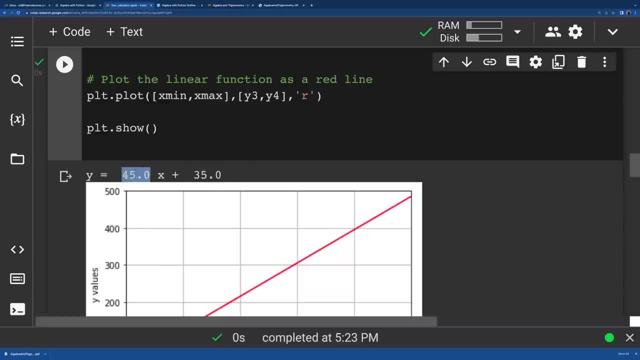 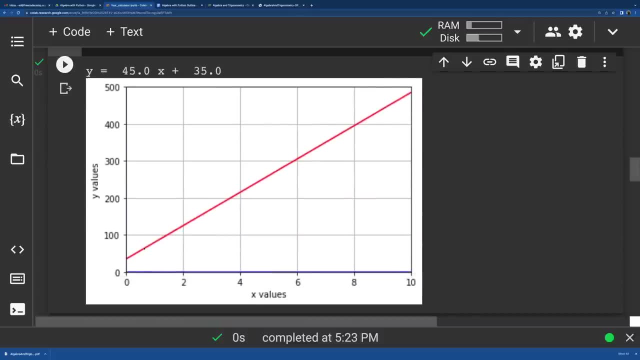 And each session must be $45.. And so we see this graph. Then you know there we go And we see the cost: 45, you know almost halfway there, And then we see the increase. Okay, somebody wants to plan. you know what it's going to cost. 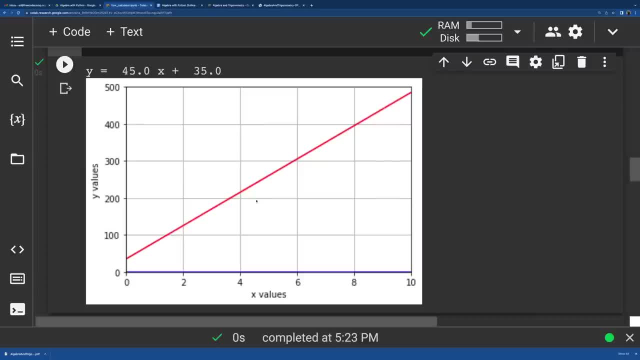 How many training sessions do I want? Maybe this is in a month. The person wants like two in a week, So it might be like you know two in a week. So it might be like you know two in a week. 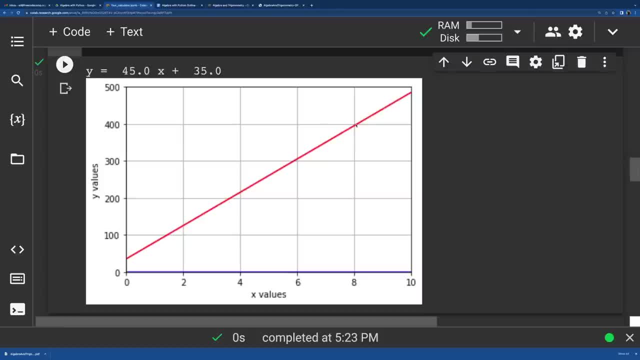 It might be about eight in a month And can calculate: oh there we go, Eight training sessions, That'd be $400.. Or, you know, do I want to just try to, you know, just pay the $35 and not get any training sessions? 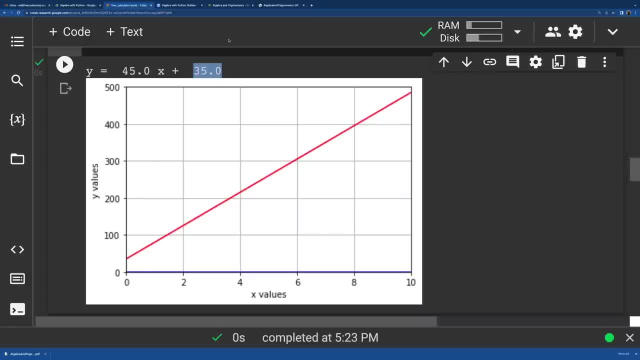 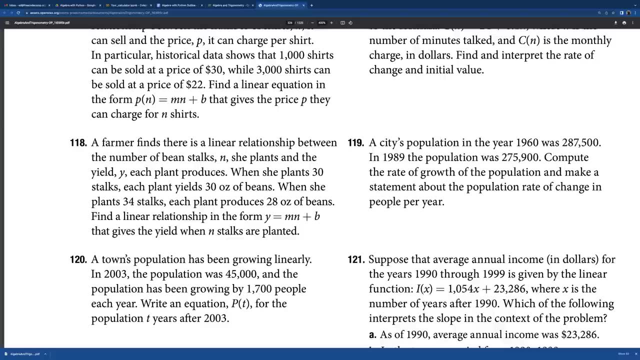 And you know there we go. Then it's somewhere around here at the zero value, And that's what we want. We want to, you know, use these to be able to calculate some different things. You know the Cost, like $116 here. 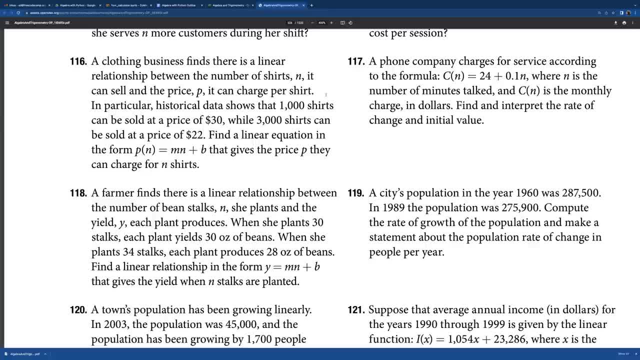 So for linear relation, Clothing business finds there's a linear relationship between the number of shirts it can sell and the price, Price P, that it can charge for a shirt. So there you go, Selling N shirts if the price is P, And this is, you know things that people want to find out, because then that helps people figure out what price. 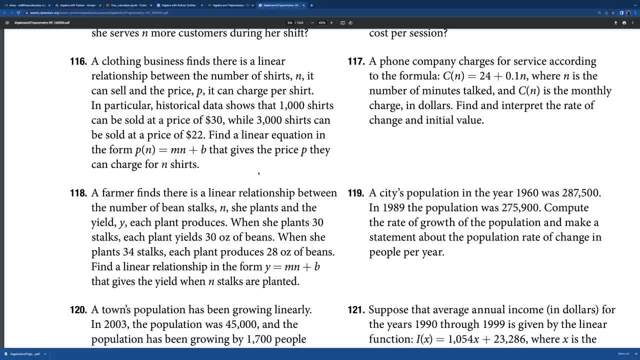 You know, they definitely start out like: can't, You know, go below a certain price because I have to make money, I can't lose money. But then, beyond that, we see, oh wow, this is shirts. All different prices are possible. 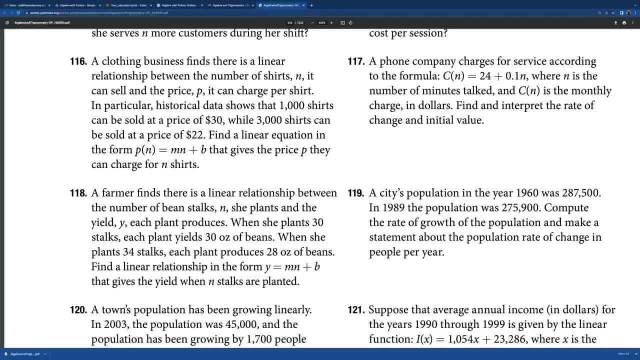 So somebody says that finds this historical data. So finding data from somewhere else. some other people selling shirts: Oh, okay, I can sell a thousand shirts if the price is $30.. But 3,000 shirts If the price- This is $22.. 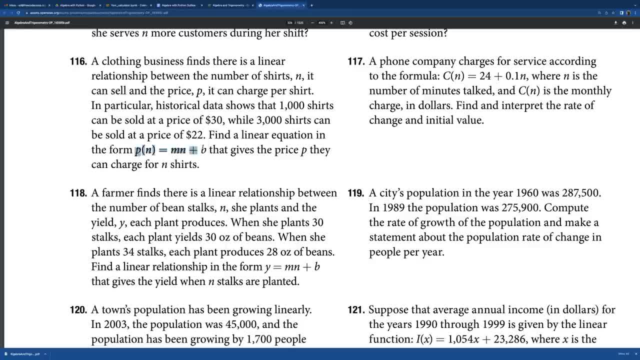 So there we go Again. that classic Y equals MX plus B, but we just changed the letters P of N. you know, the price based on N shirts is MN plus B. So there we go, We can look at this. you know N shirts. 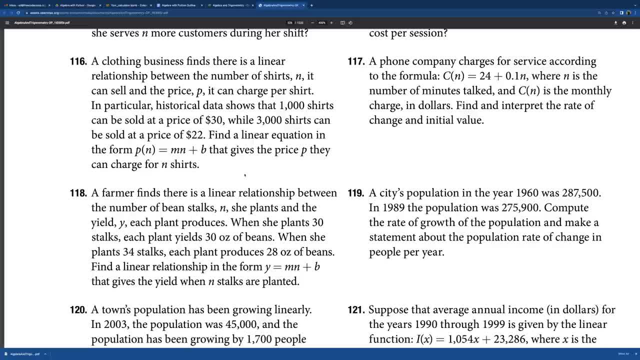 Now something like this: I might take that the price is the independent variable, because that affects how many shirts you can buy, And so we might, you know, do something like that, And then we'll get into in later units, here We'll get into other things where we can, then, based on that price, you know, given this, we can find that you know that equation for price. 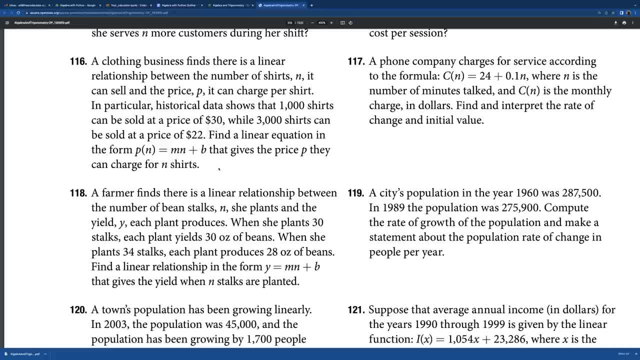 And then, based on that price, we can take it a step further and say what would be my, What would be my profit, Because, just as an example here, So a thousand shirts at $30.. So it'd be $30,000.. 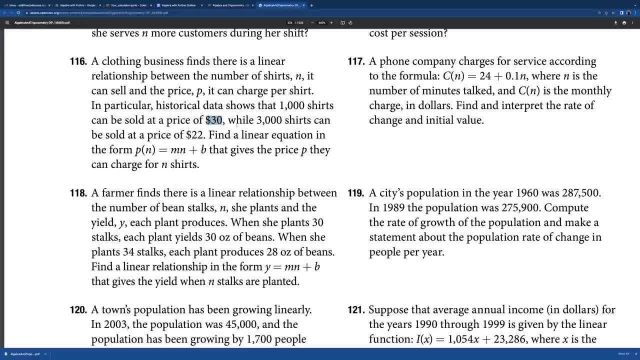 So they sold a thousand shirts $30 each, But 3,000 shirts at 22. So 22 times 3,000 is $46,000.. $46,000.. So just lowering That, not just you know, selling more shirts, but the price that it had to lower or reduce to $22, not that much different. 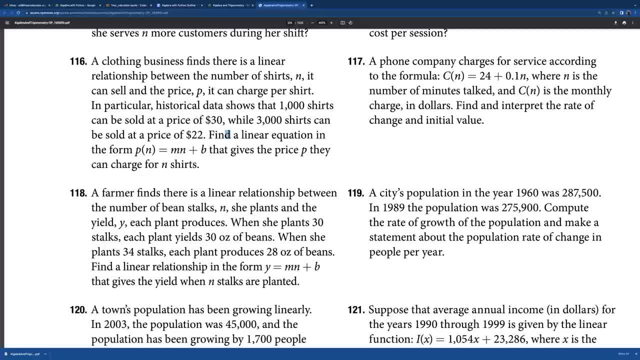 And so it sells 3,000 shirts. So instead of $30,000, $66,000, look at that- all more than twice the profit for a little bit less, And some people who don't look at the math of this would say that. 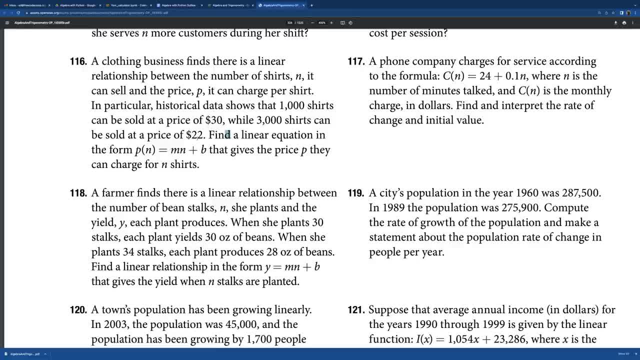 You know, is the, you know, reducing it $8, is that going to double my profit? Actually it does, Or at least the revenue. We don't know the cost of making the shirts, But it more than doubles the revenue. 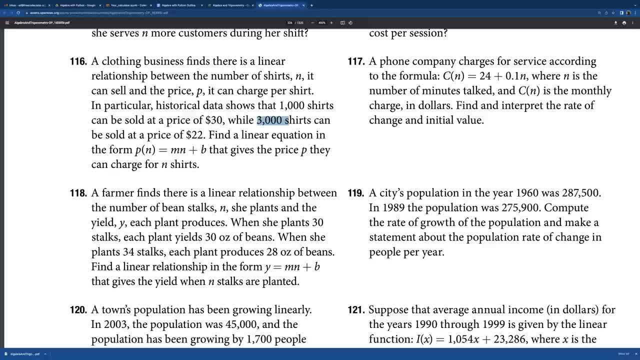 Just lowering that a little bit because it reached so many people, And so that's what people are looking at. you know- And again in further units we'll look at the math behind- you know how to get this, How to find that. 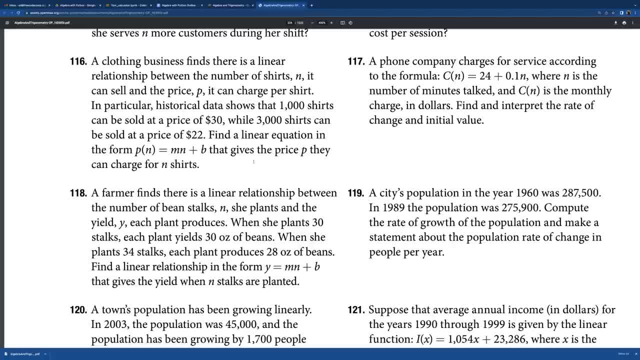 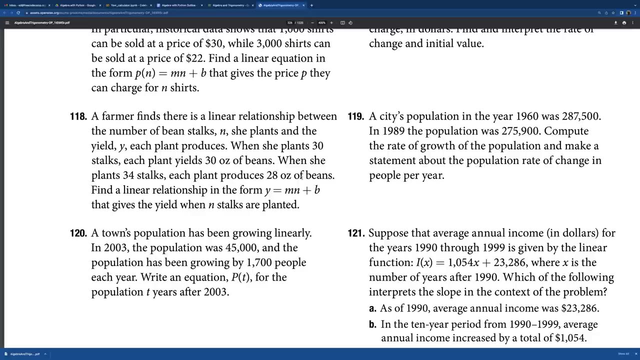 Maximum profit value, Maximum revenue value, And you know what are we looking at here. How can we find that ideal shirt price? So there we go, There we go, All of these others, Same situation, Linear equation. We're trying to maximize things. 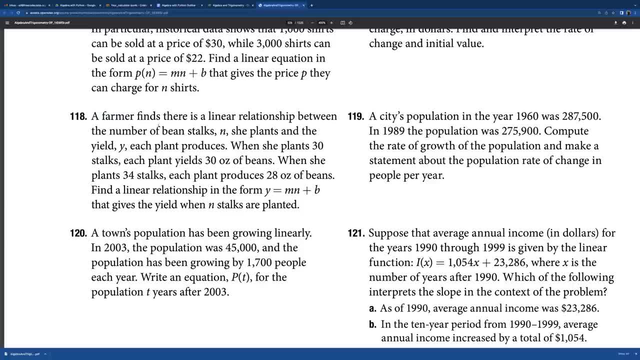 If we look at number Number 18 of a farmer finds a linear relationship between the number of bean stalks she she plants and then the yield that each plant produces. So 30 stalks Each plant yield, you know how many per per acre. 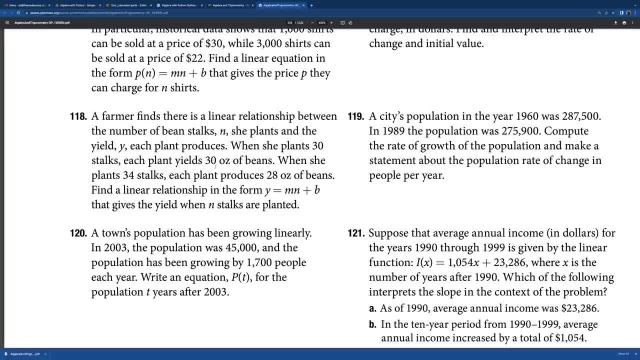 So 30 stalks Each plant yields 30 ounces of beans. but then 34 stalks reduces it to 28 ounces of beans. You know they're all competing for some of the same resources. So we can definitely get that linear equation and then we can try to find. so what would be the maximum? you know how? what would maximize the bean yield? 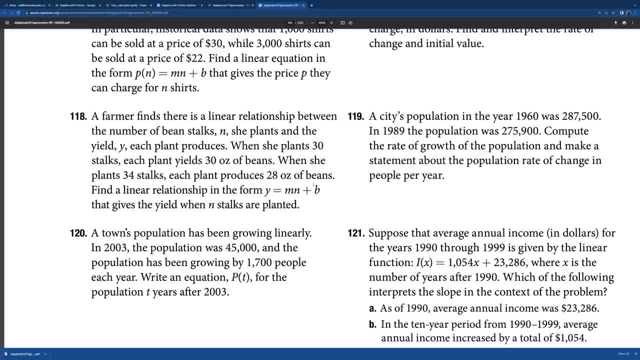 So you know it'd be really interesting. So Then we get this- Yes, so notice this- And the yield would be 30 ounces. 30 ounces Ounces: that many beans times 34.. Oh, no, sorry. 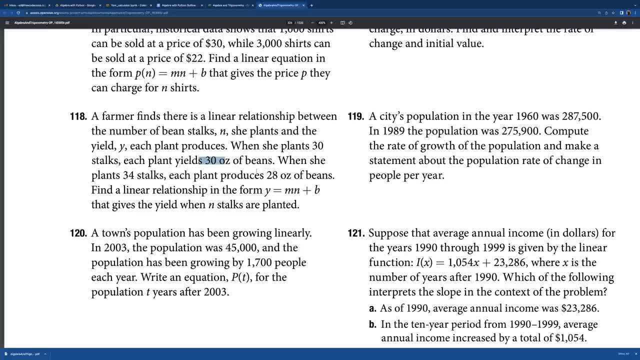 30 stalks times 30 ounces- See then 30 times 30, so that's 900, or then we have 34 times 28.. And I'm not going to do that in my head, but we can see some different values and then we'll look at these in some of the other business applications. 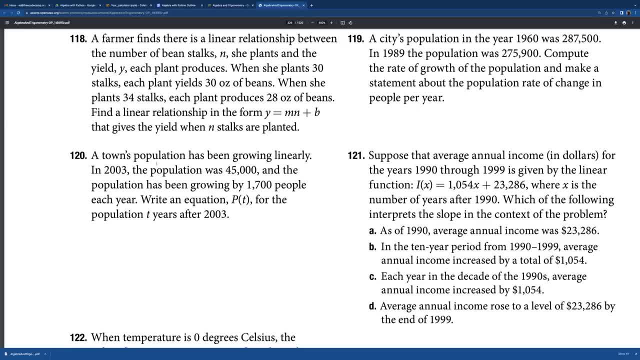 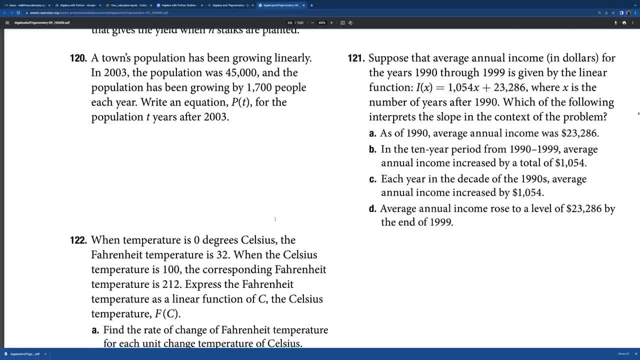 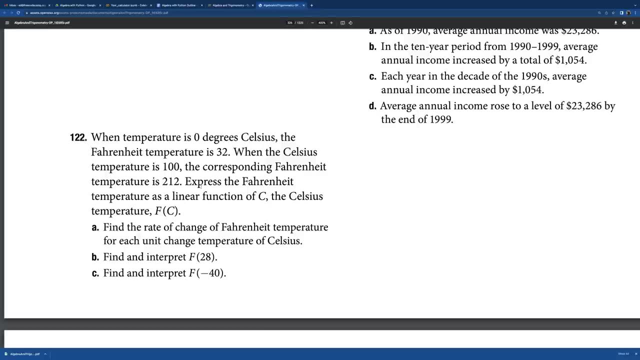 Later on. so some more things. if we, if the town population and like number 120 growing linearly, we can write an equation for that, You know. here's another one where We often do this all the time, converting temperature from Celsius to Fahrenheit, and we have these two values. 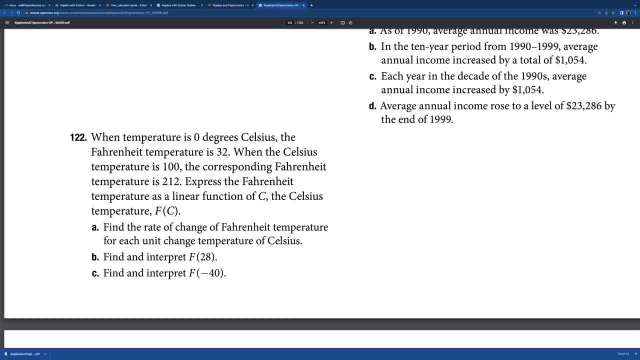 Zero degrees Celsius is 32 degrees Fahrenheit. So Then we know, A hundred degrees Celsius is when water boils, and the corresponding temp is 212 Fahrenheit. So what you can do is we can just take these Now. we could also use this to make another function. 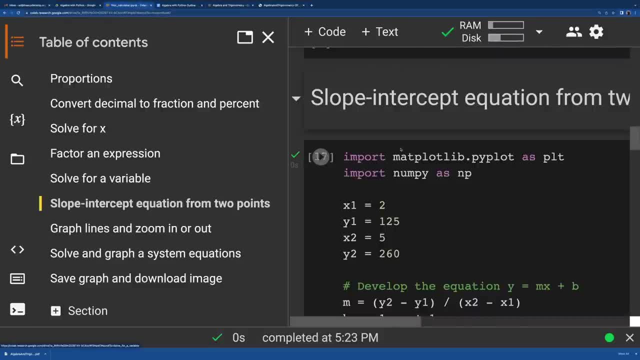 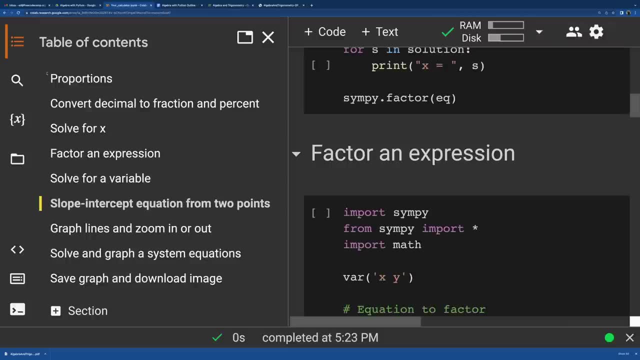 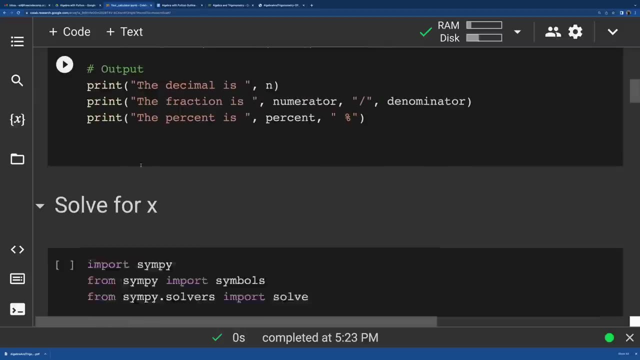 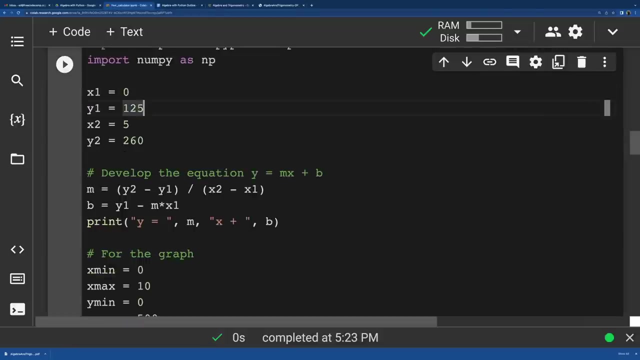 But we could also take this, you know, slope intercept from an equation, Equation from two points, and There we go. So, but except equation from two points, And We can say: All right, so we have zero and then 32.. 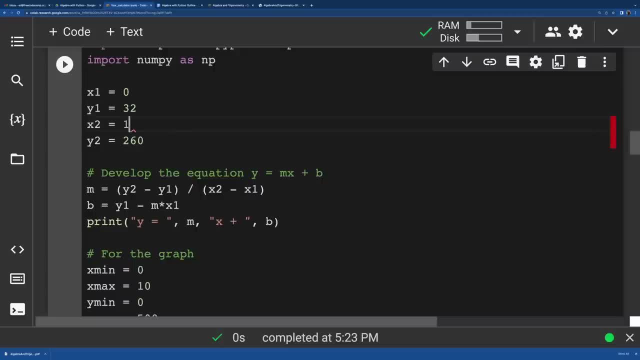 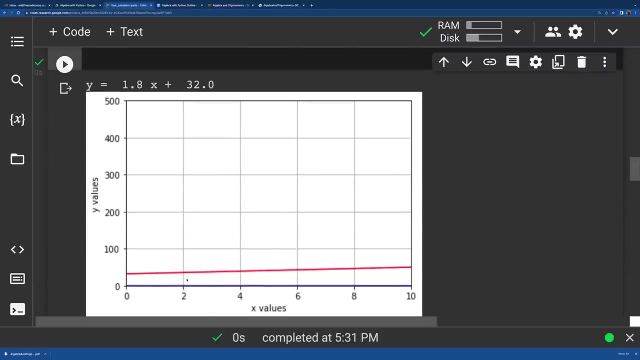 And Celsius would be a hundred and Fahrenheit be 212.. Yeah, and see the See the graph. Now the graph in this case. okay, and I'm not even worried about changing the values, because the main thing we wanted was this equation here: 1.8x. 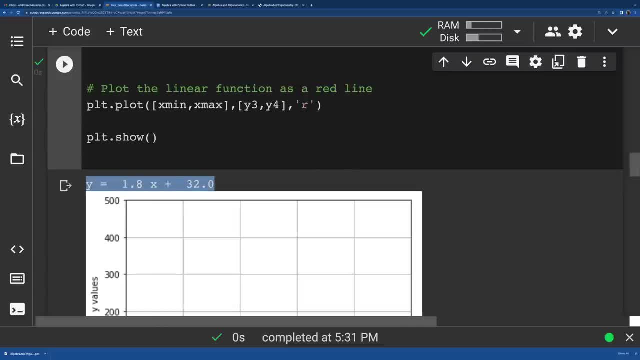 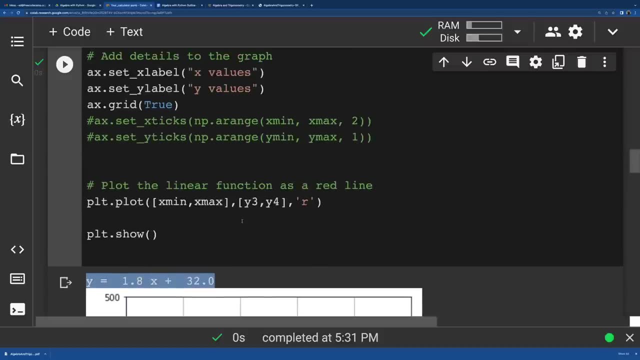 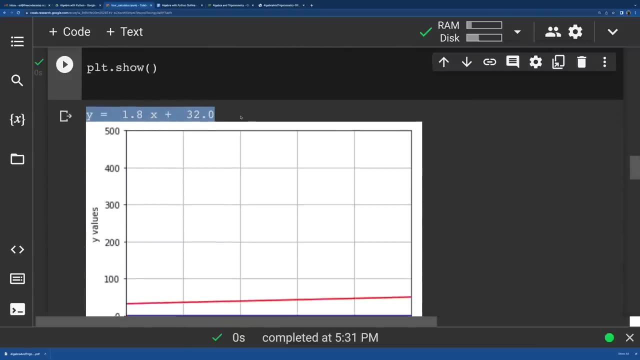 minus 32.. Some people like that. 1.8 is a fraction, it's 9 over 5.. So there we go And remember. then the x value was Celsius. so that's how we can convert Celsius to Fahrenheit Times: 1.8 plus 32.. 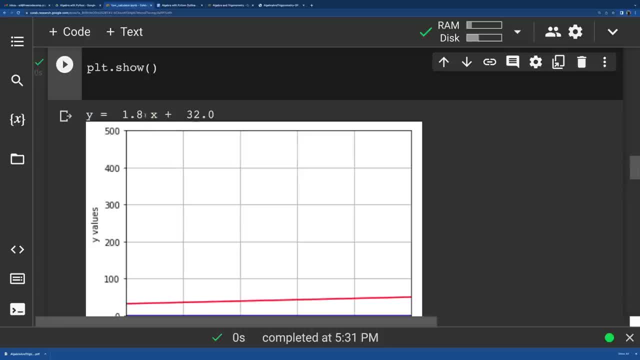 And so if we look at the increase, you know 1.8 is almost 2, so you know each Celsius degree increases almost 2 degrees Fahrenheit increase. So we can see that change. So if we take a look at this, 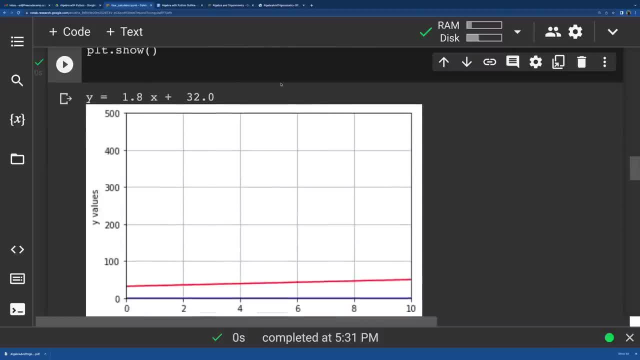 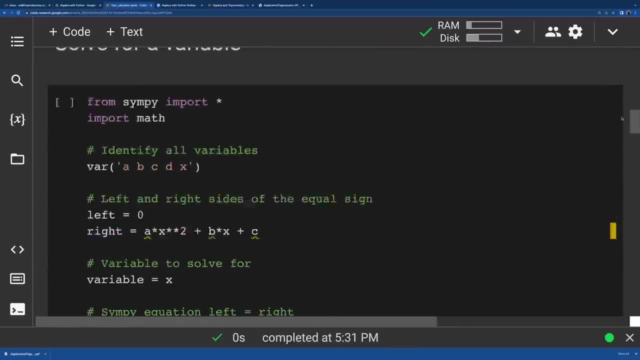 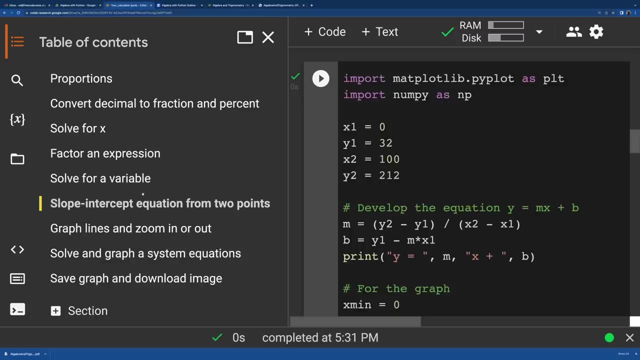 you know you could always make this, that you know. make another function for yourself that you could. you know you could just have, like you could just have Celsius to Fahrenheit, Fahrenheit to Celsius, you know. then make another section. 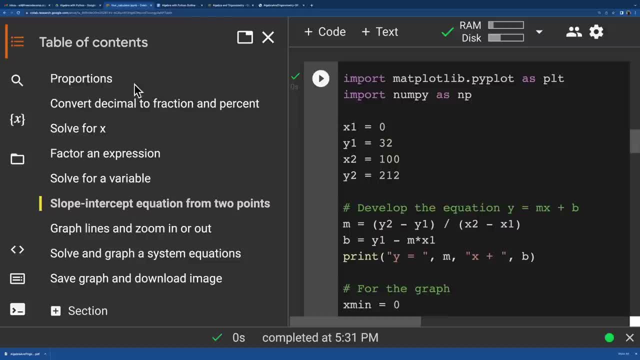 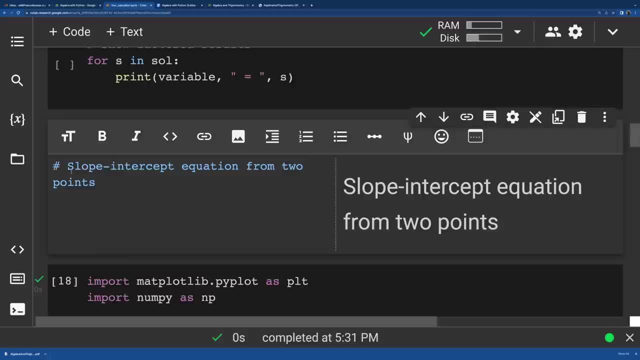 add it, you know, put a heading to it, because, remember, as soon as you have the heading, you know, not a comment, because we're not in the code, but if it's in there, then it becomes a heading and it'll be, you know. 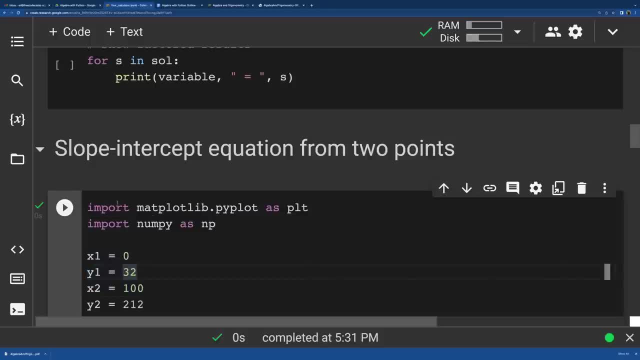 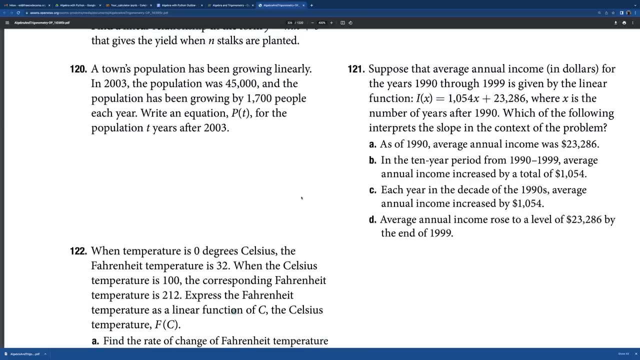 be in the table of contents So you can always make some of these things for yourself And you know, that's why I want to give you some of these practice problems, You know, if some of these are relevant or if you want to combine some of the things, you know, you have room to. 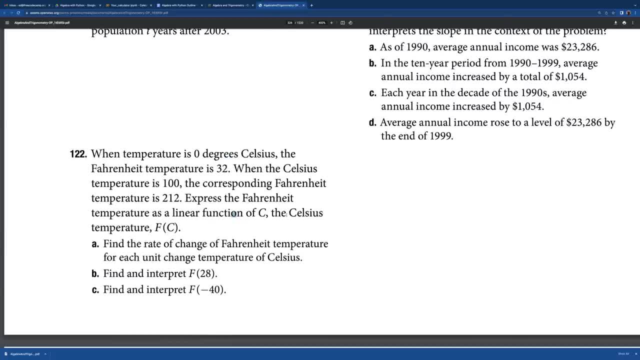 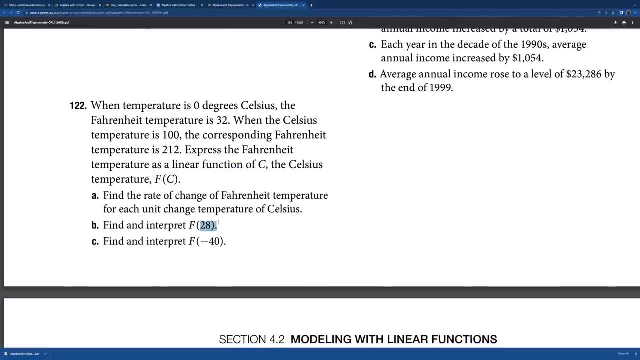 explore and do some different things. So there we go, And then once you have that equation, you can find- you know, there you go- that function of 28 degrees. what's that become? in Celsius, or in Fahrenheit, or negative 40. That's a good one, Because negative 40. 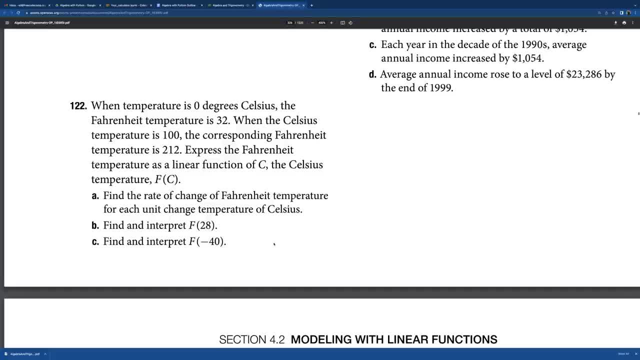 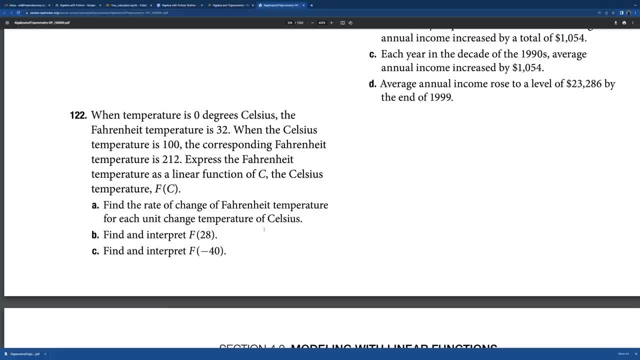 Celsius is negative 40 Fahrenheit. So the one time where they actually agree It's got to be really cold. But when it's that cold they agree And anybody not even having a thermometer would probably agree to: yes, it's cold. 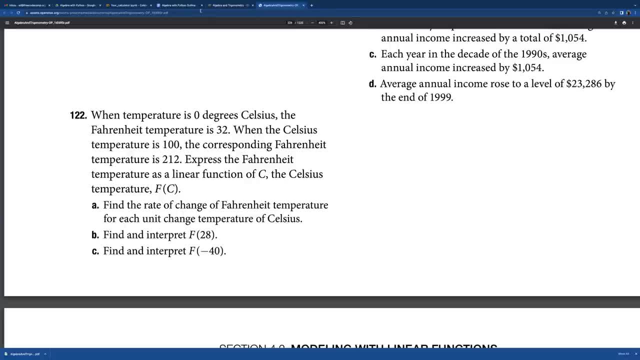 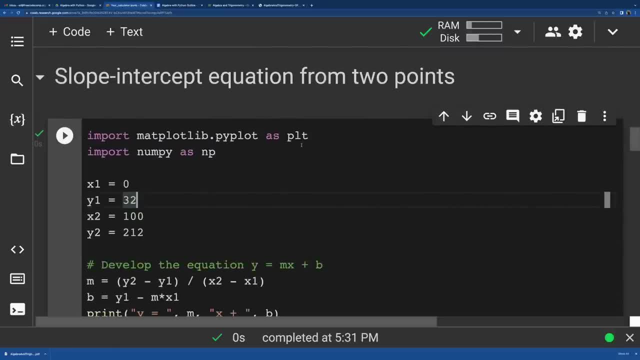 So these are some of the things applying, some of some of these- And hopefully this is you know for find this useful- some, some ways you can interpret some of the word problems and use some of the notebooks that you've been working on to solve problems. answer questions. 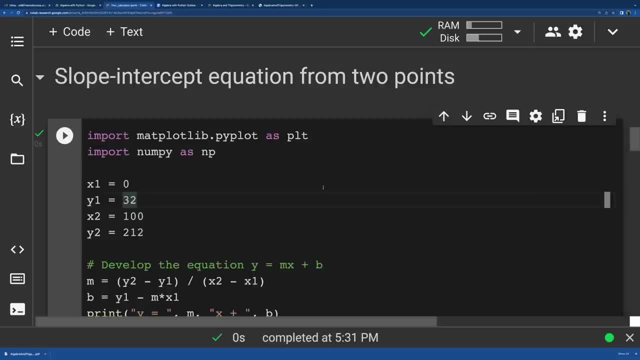 And, yeah, you can continue. you know, add more to what you have. you know, make, make it your calculator. Anytime you have different formulas, they say, Oh, this, this might be useful. make a function, make a formula, another notebook section. All right, ready to go on to the next. 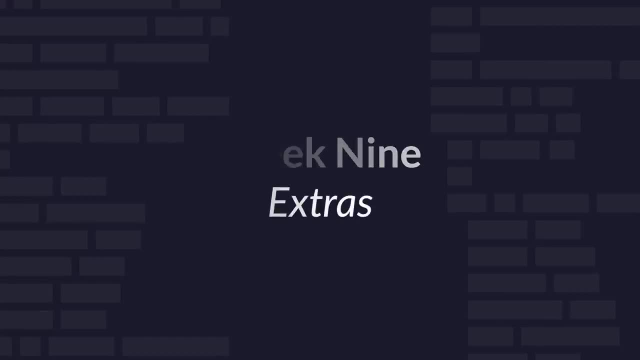 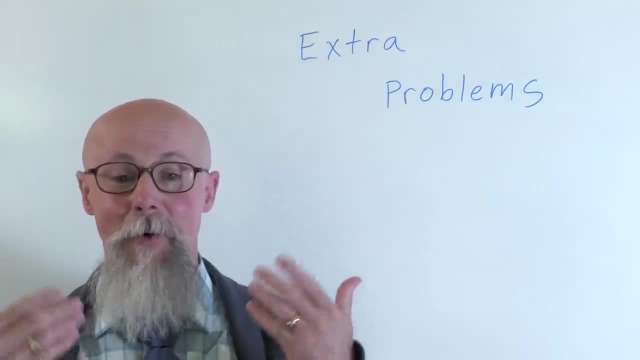 thing, Now that we've worked through the core skills in this unit, let's look through some extra problems, And I'm going to work through extra problems using the Colab notebook So you can see how you can apply these resources that you're building. 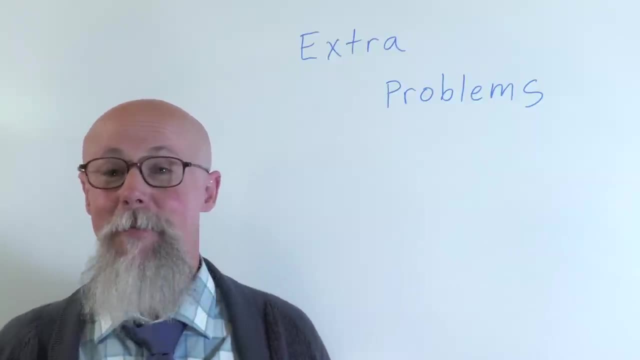 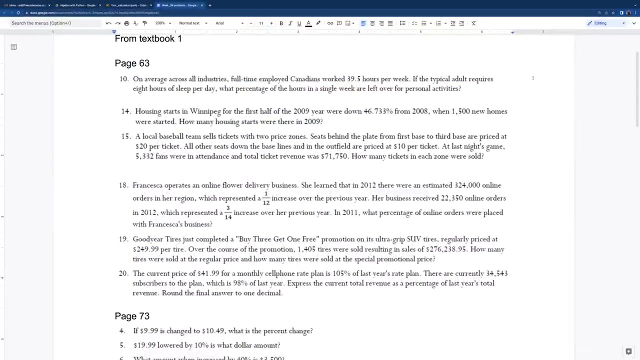 And use the use these to solve problems that might come up in a textbook or in day to day life. So we're gonna go through some more extra problems here. For these extra problems, we're gonna look at just ways to set up some formulas. You know, if you have different situations, word problems, 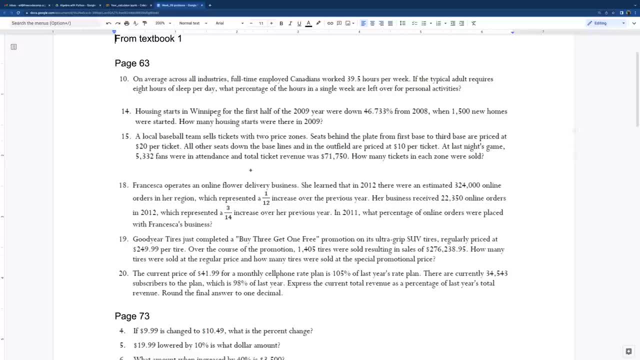 how can we decode these, put them into math terms and then use Python to solve them? So just here's some examples, And all these come from the pages in the first textbook. you have the link. So let's look at number 10.. On average, this happens to be full time. Canadians work 39.5 hours per week. So if the typical 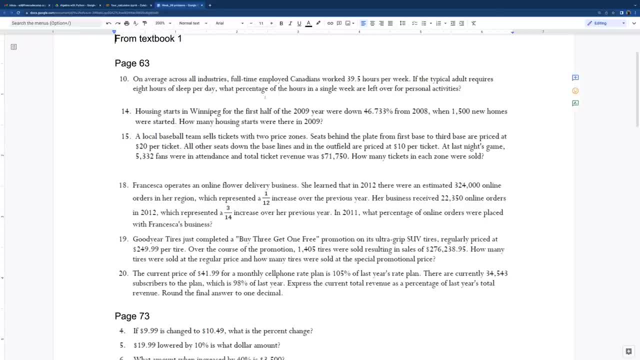 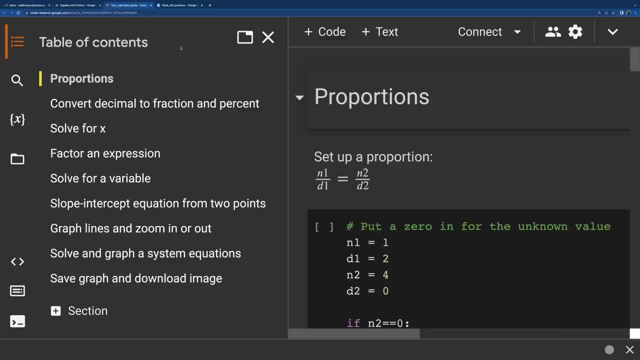 adult requires eight hours of sleep per day. what's the percentage of hours in a single week left over for personal activities? So we need a few things here: 30.. So we need the number of hours in a week. And even just going through your Python collab notebook, we have all these different things that you can do. 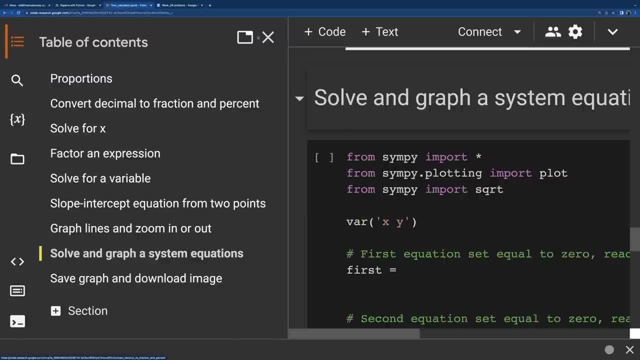 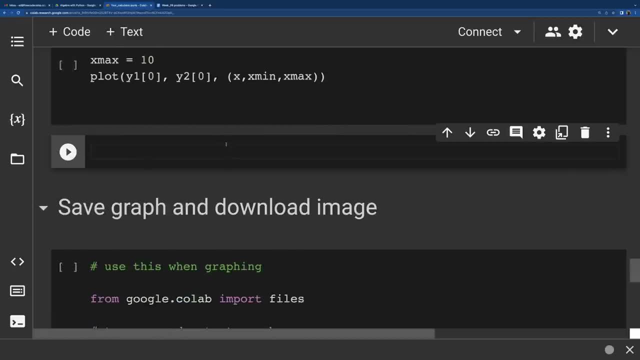 I'm going to click on solve and graph, which we're not doing yet. But in here you can just put a blank line of code. here, And even in the print statement you can do a lot of math. So first of all, we can 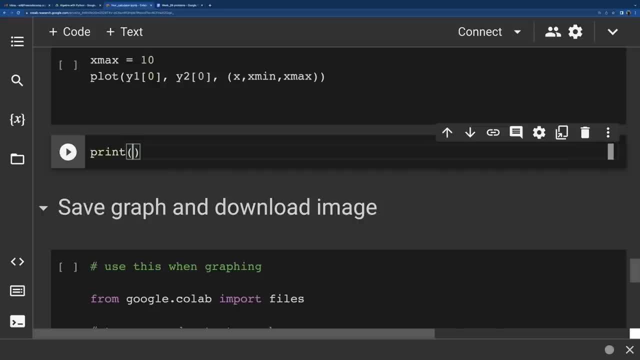 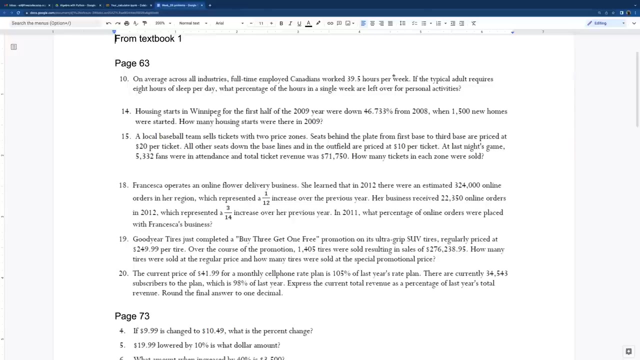 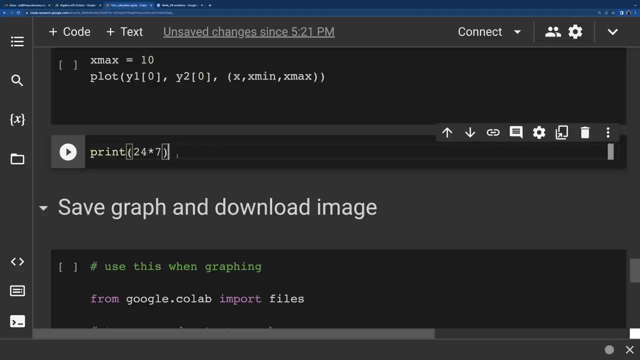 have the number of hours per week, and that would be 24 hours times seven days. and then if we want to look at the number of hours that Canadians work, we're going to subtract 39.5 from that, and Python knows the order of operations. so I can just put in here: I like the. 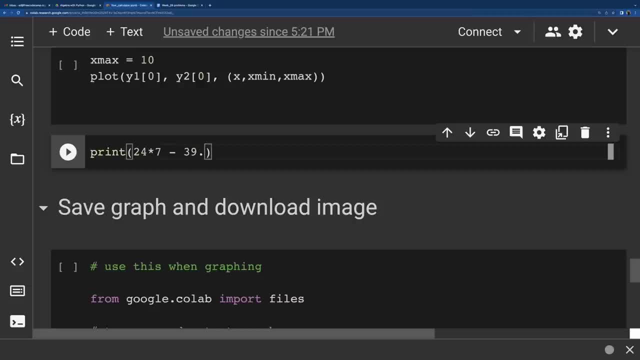 spacing, but you really don't need it- 39.5. so there we go: 24 hours a day times seven days a week minus 39.5, and then we actually can also subtract eight hours a day eight times seven. so we have how many total hours in the? 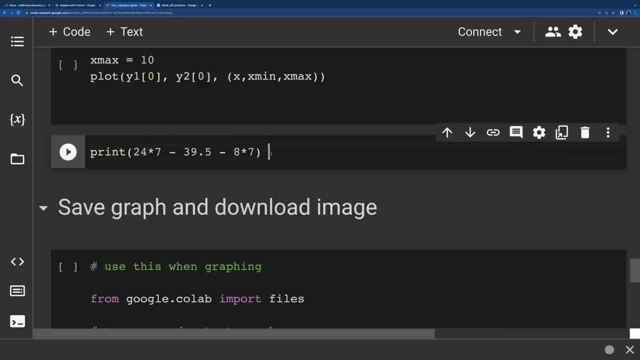 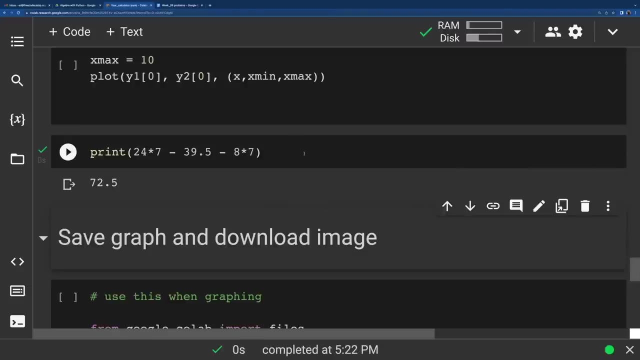 week, and then minus the work hours, and then minus the sleep hours, again all this in in Python shift enter and we will have seventy two point five hours. so there we go. seventy two point five hours is you know, and it works out. look at, look at that. you know. work, sleep still have plenty of time to go. 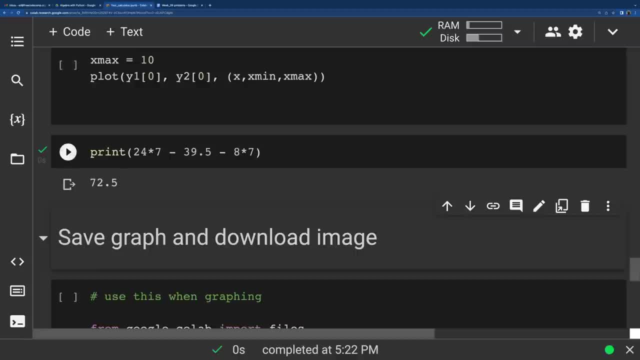 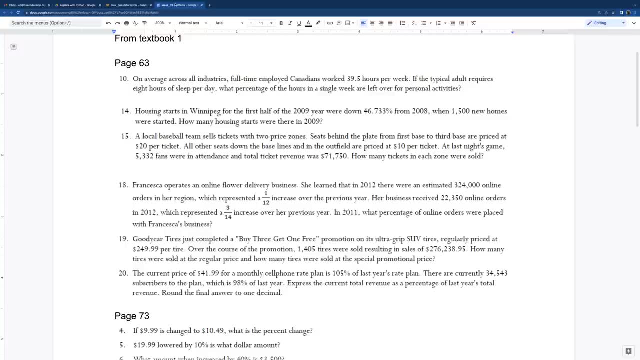 out and do things, and we can do all this- just know knowing what we need to do each step. you can break this up into different steps and put variables, but this is just one way to do this. all right, and let's take a look at another one: the number 14 housing starts in Winnipeg for the first half of 20- 2009. 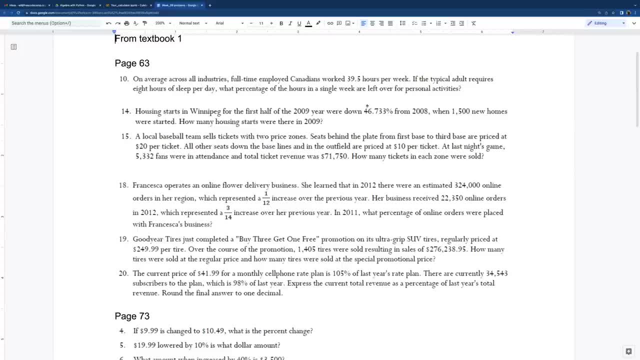 we're down forty six point seven, three, three percent. we'll talk about converting that in a second from 2008, when one thousand five hundred new homes were started, so from 2008 to 2009. if it was the same amount, it would be that times one or times a hundred percent, which would be times 1.00. so if 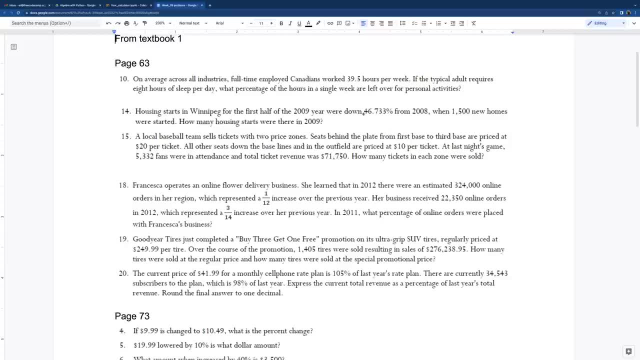 it didn't change. it would be that times one. but then, since it went down, we want to think one minus that rate. so it's not the hundred percent, it's the hundred percent minus this forty six point seven, three, three, and then we're down to the. 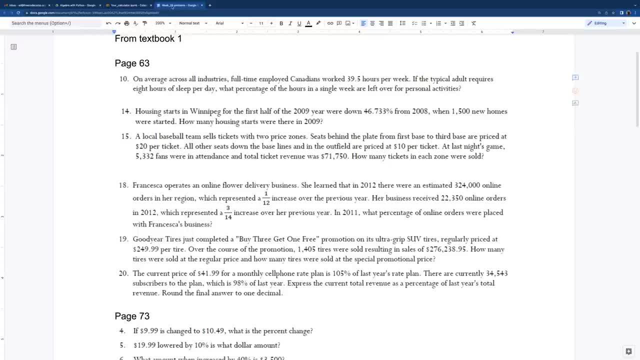 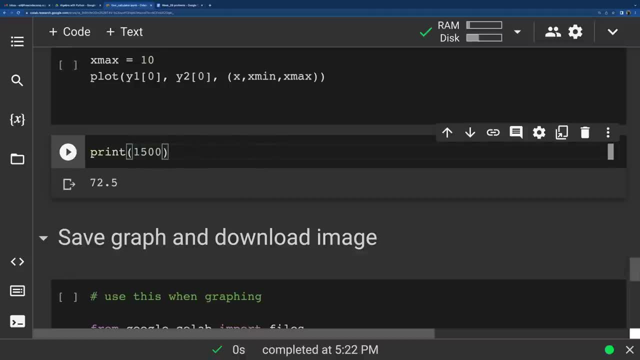 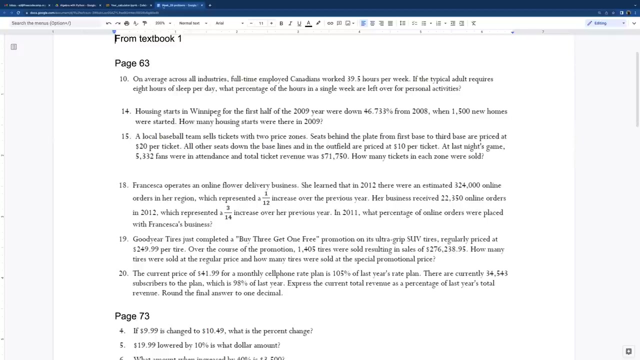 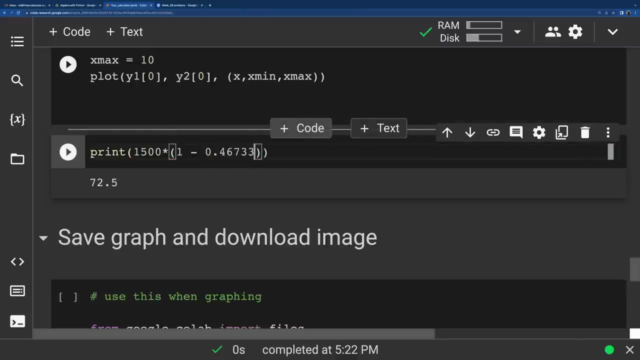 the original was in 2008. it was 1,500 new homes. So we can just go right back to this and we have 1,500 new homes. times 1, minus that 46.733 as a decimal is going to be 0.46733, and you see that we have that, that decimal. so 1 or you know. 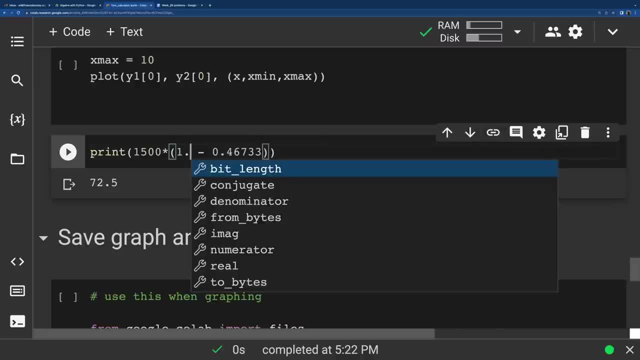 100%. I mean it's not gonna mess up the code if I put 0.00. we don't need to. but so you know that's a hundred percent. so if it was that 1,500 times 1 that would be, it would not change year to year and since it went down it's. 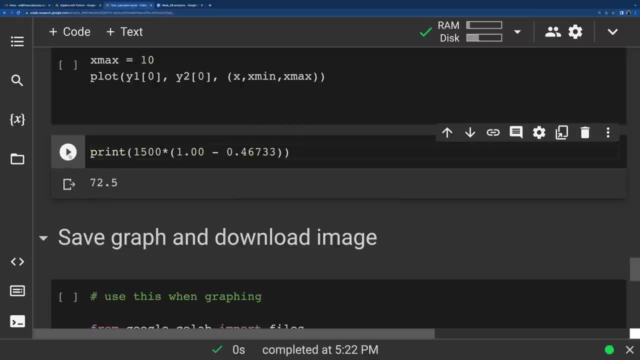 times 1 minus this rate. you know this will just overwrite this and these are number of homes. so we're gonna round it down and we're going to say it's 799. you know that point 0, 0, 5 is. you know that's what five thousandths. you know, I don't know, they put a few. 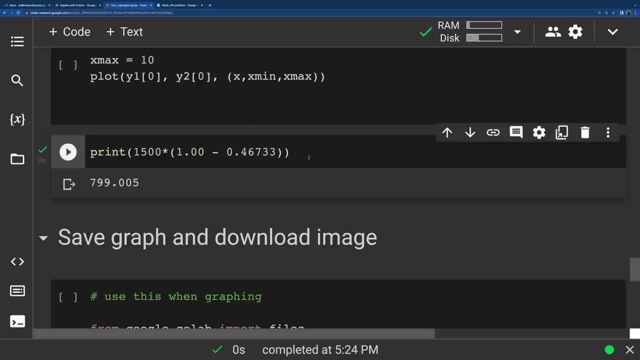 boards there or something on the lot, said I started, but there we go. we're going to call it 799 and that's how we get this times, you know, minus the rate since it went down, And in later weeks we're going to talk a lot more about percent. 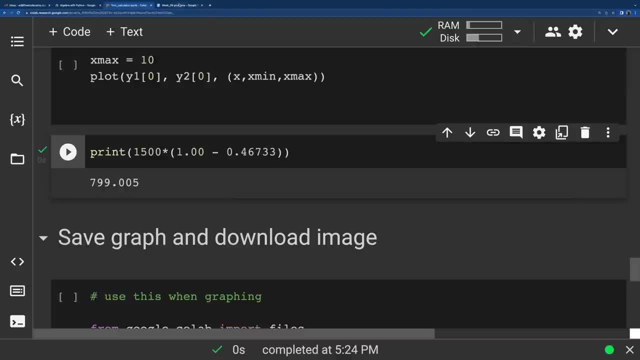 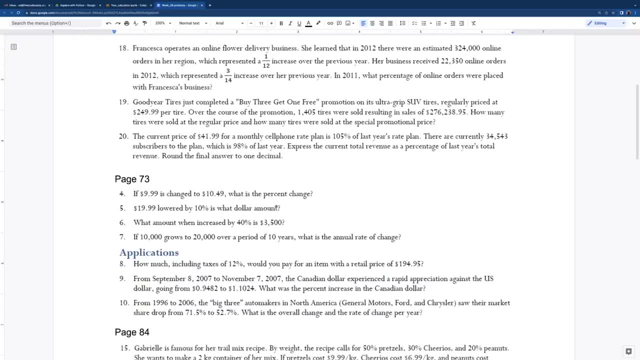 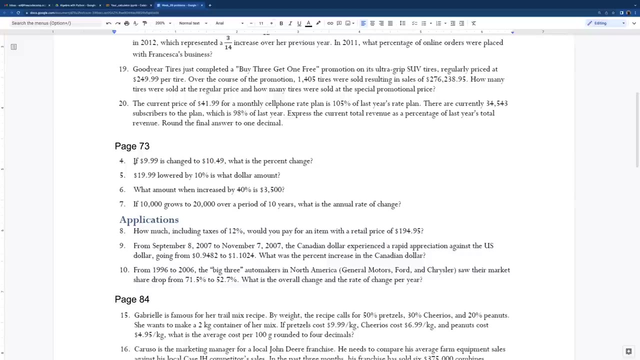 increase and decrease. So this is not the only time you're going to see this, And in that case we're going to skip some of these other percent increase or decrease. But on page 73, I want to talk about this percent change. So if $9.99 changed to $10.49, so the amount of change. 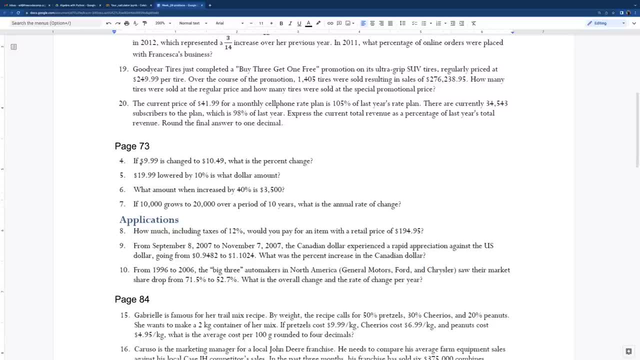 we would just subtract $10.49 minus $9.99.. And we see- you know, we can do that, You can do that in your head It's an even 50 cents. But then the percent change is. we take that difference. 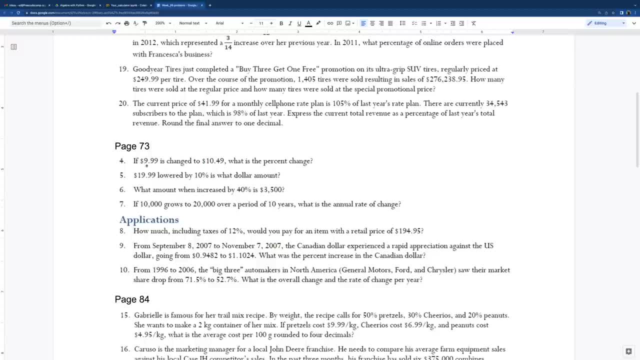 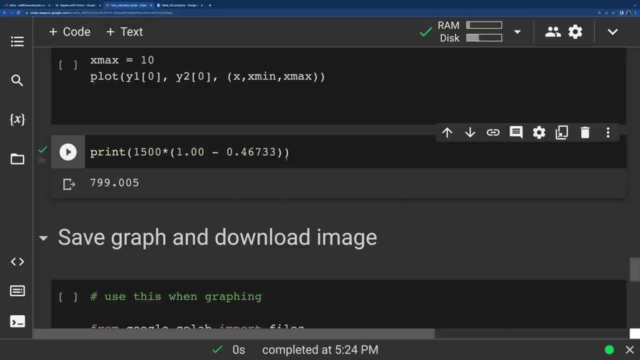 over the original number. So if it started at $9.99, that's the difference, So that's the original number. And again we can look at percent change So that 50 cents 0.50, divided by that original number, 9.99.. So that's, we get that difference divided by the 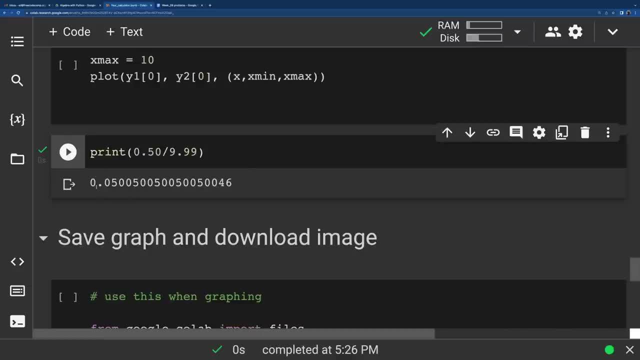 original number And as a percent, we're going to multiply it by 100, because it's the first two digits And even if I were to round it, the next number is a zero. So it's really a 5% change. There we go, And if you really wanted to, sometimes people like to put that into the 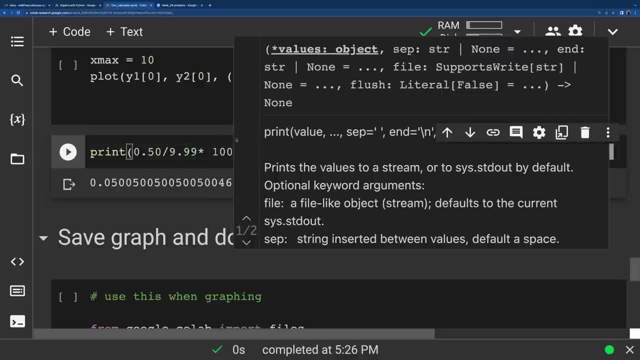 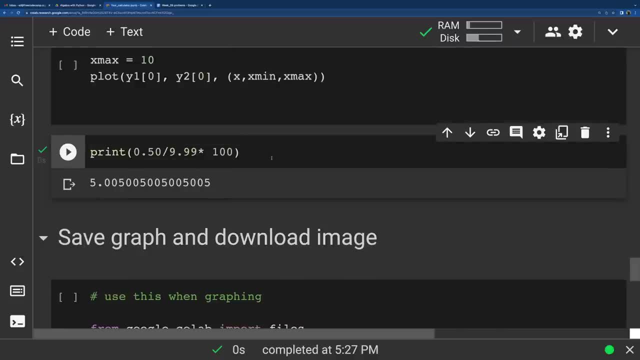 formula times 100.. And yeah, there we go As a percent. I mean, if it's just for your own calculations, you don't have to make it fancier If you're doing this to explain costs and everything in some sort of business proposal. 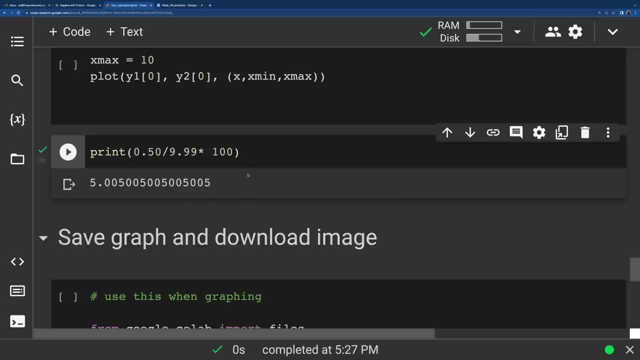 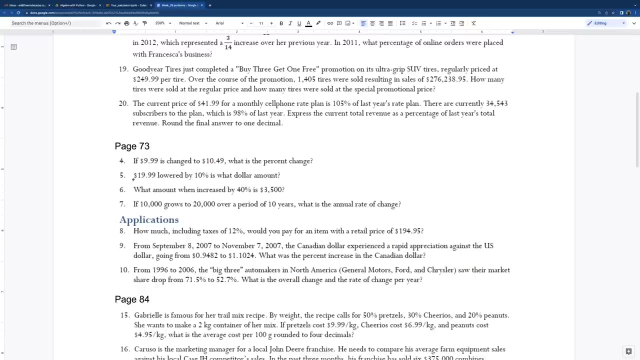 yeah, it's nice to have the extra bit, have it display nicely and people can see: oh, this is exactly what you're talking about For your own calculations. you can put it all in the print statement and see the output, And there we go. So if we have $19.99 lowered by 10%, 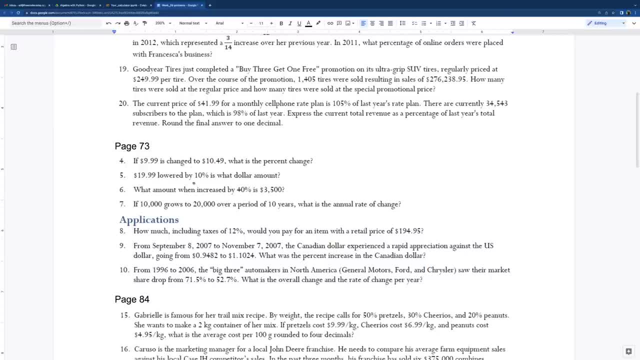 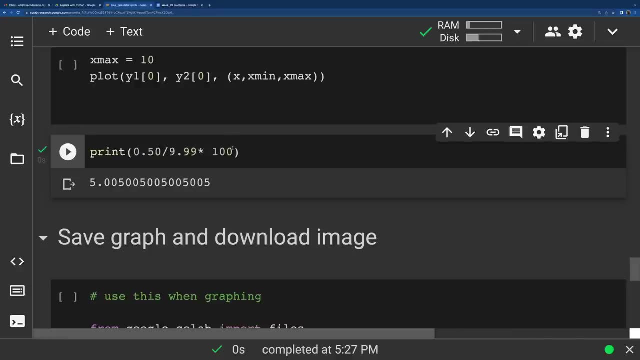 so we're looking at these keywords lowered by, and if it's a percent we need that formula one minus the rate. Again, might be new to think about it this way And we're going to talk a lot more about it in later weeks. But $19.99 lowered by 10%, So we're not decreasing by an amount, so we're not. 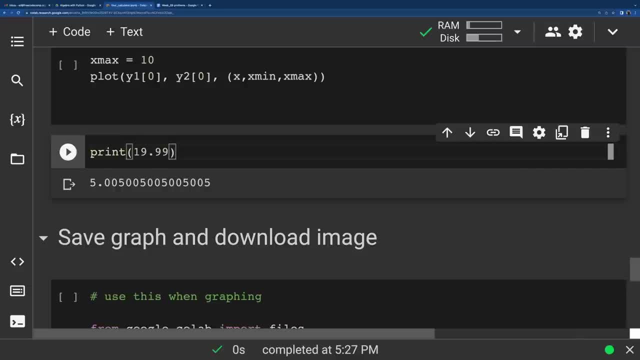 subtracting, It's times one minus three, And I can even, you know, convert this, as I'll just put this here: one minus 10%, Remember 0.10.. So I put that in there with the extra zeros. But you can see that that's where. 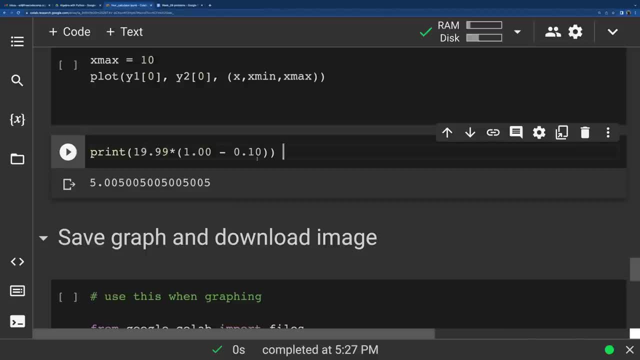 we get this one minus three. If it didn't change, it would be that number times 100% or times one, But it's times one minus three And then that's the new number. There we go, And this did not have any practical connection. It was just what's the number. 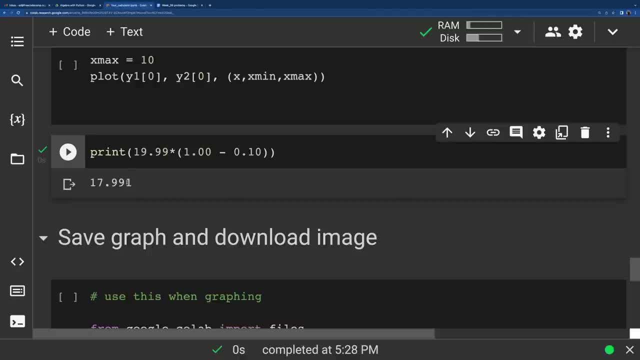 If it's a dollar amount, then I'll take it to two decimal places: It's $17.99.. So that'd be something like: you know, the shirt cost $19.99, and it was on 10% off, So you end up. 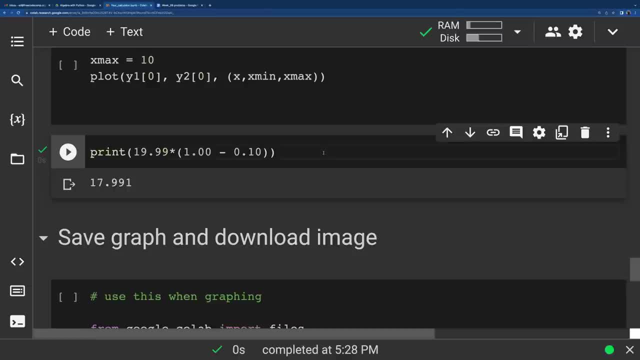 paying $17.99. And knowing how to do these things. you know we have a calculator So you can do this right there on your phone Because you can have this app. You can set up different things for percent increase and decrease And you know you're in store. Oh, what would the actual price be? And at that point, is it worth it? There we go And here we have this. what amount, when increased by 40%, is $3,500.. 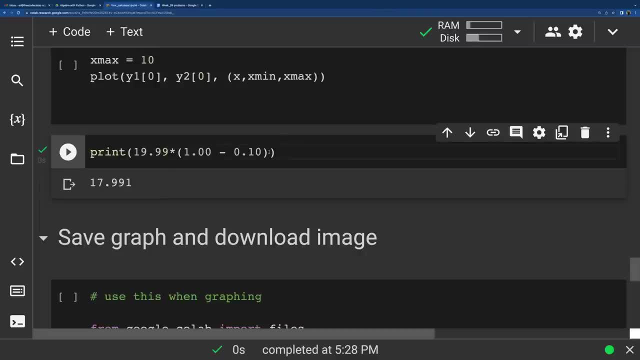 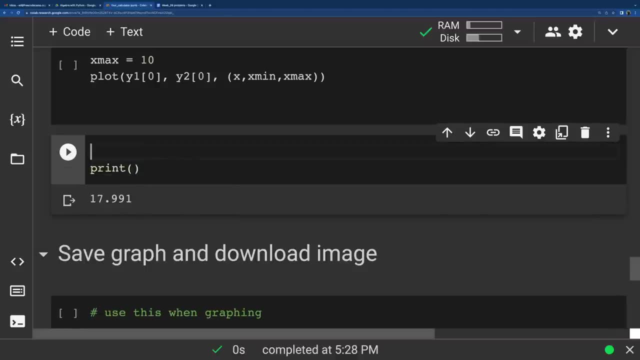 Now for this. before I even get to what we're going to calculate, I'm going to put a couple of comments here, because I don't want the code. I just want to show you the math of this. If I have some amount, which I'm going to call X, increased, 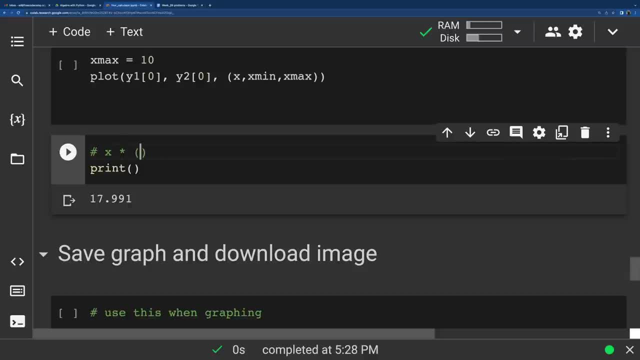 by 40%. So if it increased then it's times one plus the rate, and then that would equal that new amount. So you know the beginning amount, or you know X, or we can call it the original amount. 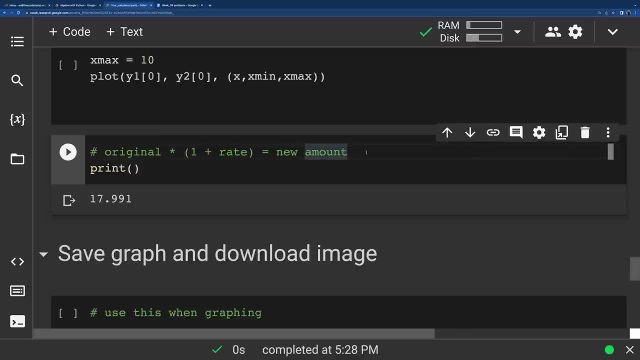 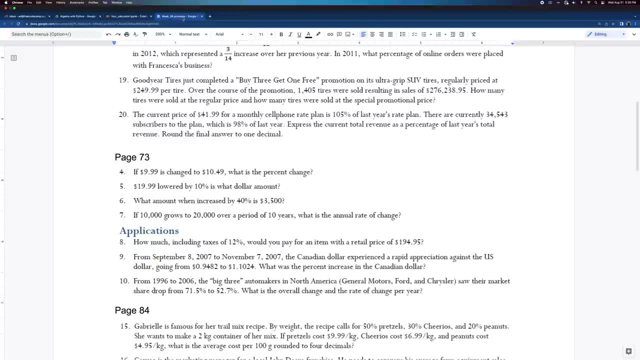 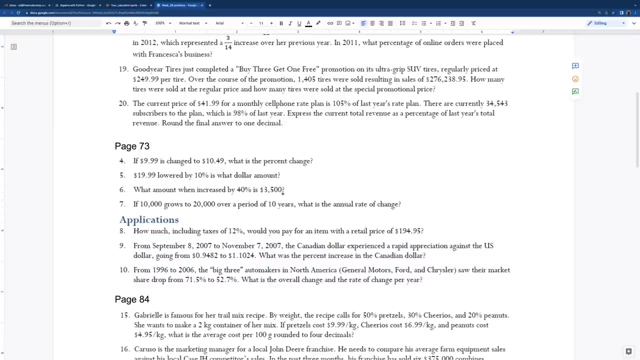 times one plus three equals the new amount, And I just put this in a comment. we're just looking at this formula And so if I have this, then the question is: what amount? number six here, what amount when increased by 40%, is $3,500?. 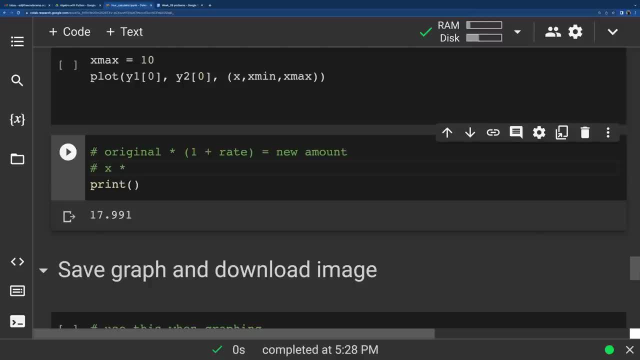 So that would be X times, and when it's 1 plus 3, that makes it really easy because it's 1.4. I put the 0, if I wanted to equals 3,500, because 1 plus 0.40 is 1.4. And then in doing this we remember solving. 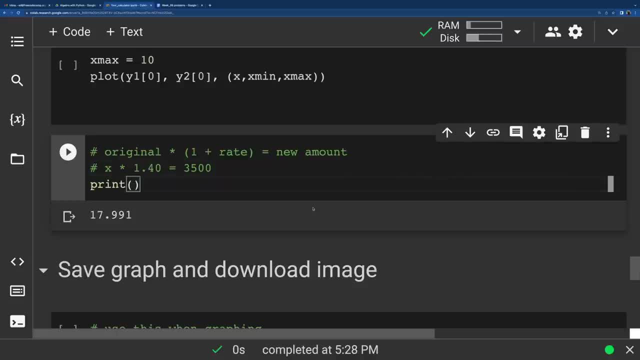 for x, I'm multiplying, so I divide, and now really in the print statement I'm doing this: 3,500 divided by 1.4. And we see how, in setting this up, you know you could write your math in. 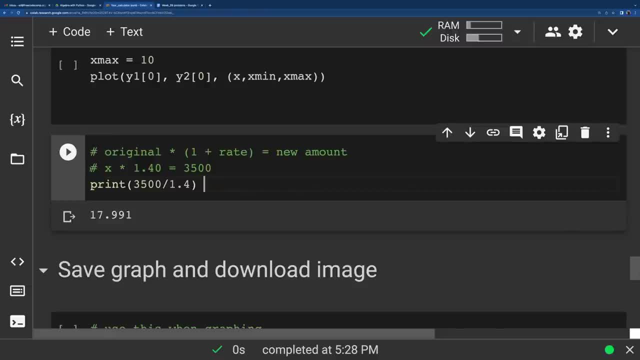 here some notes for yourself, the formula you're using, and then plug in the numbers, so then we see what's the actual math that we're doing And then dividing by 1.4, so we'll do that and that's the one thing that will print the other comments. There you go: $2,500. 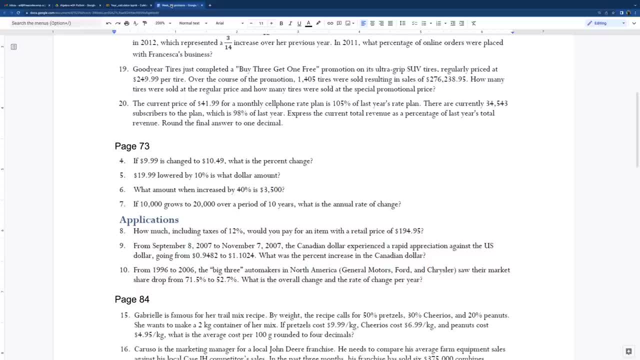 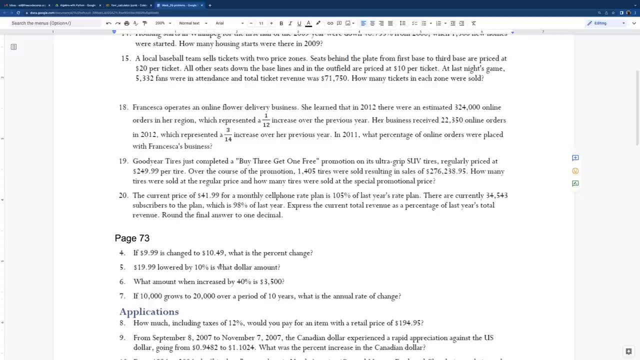 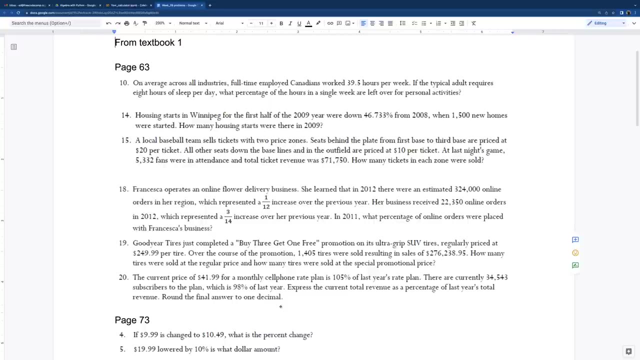 So we have some of these, All right, and I actually want to skip over to this baseball one. I skipped over that because I think those others are more straightforward. Now let's take a look at making use of you know, as you're building these, this notebook for yourself. let's make. 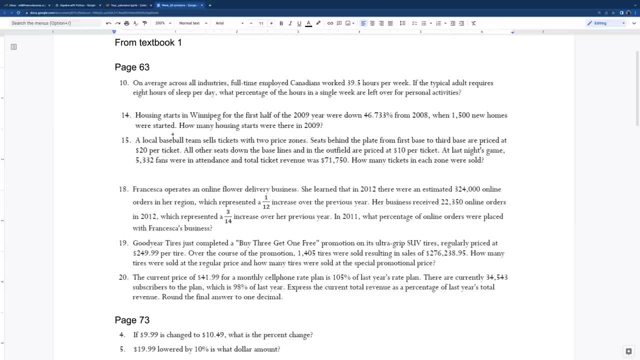 use of the system of equations one. So if we look at the system of equations one, we have a number 15.. The local baseball team sells tickets with two price zones. Seats behind the plate from first base to third are priced at $20 per ticket. All the other seats down the baselines 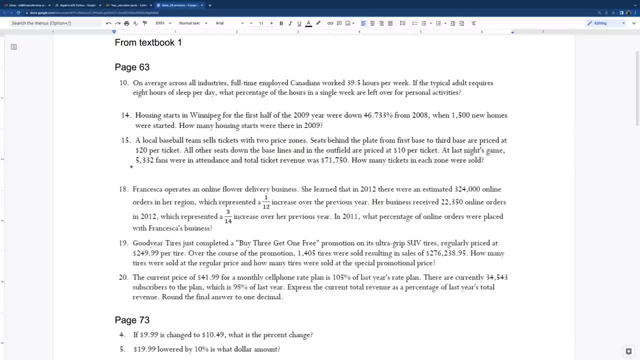 are $10 a ticket And last night's game 5,332 fans were in attendance and the total ticket revenues were 71,000.. How many tickets were in each zone? So let's call x the good zone behind home plate. Those are the $20 tickets, And let's call y the ones that are 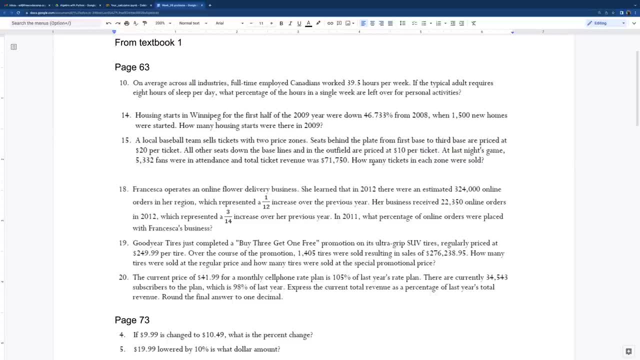 further out. So we have the two things. we want to know How many tickets in each zone. So let's think about equations for this. So $20 for the good tickets, $10 for the lower price tickets and the revenue is 71,750. 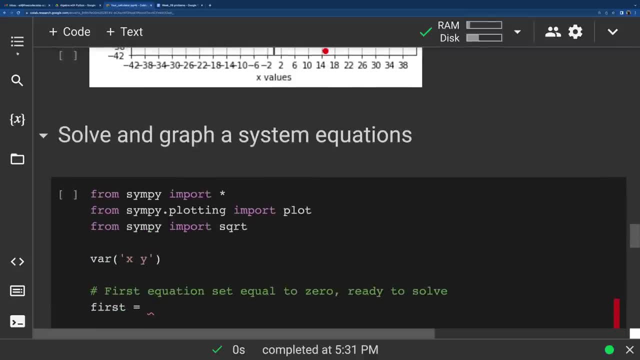 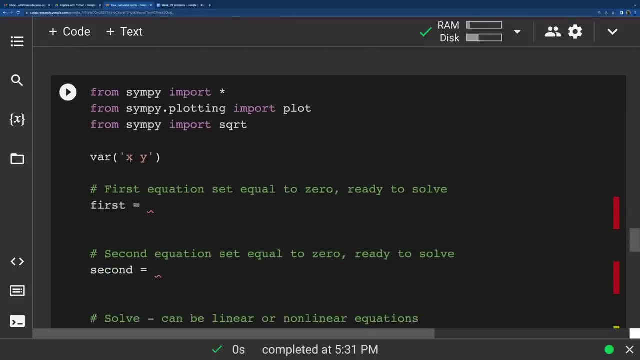 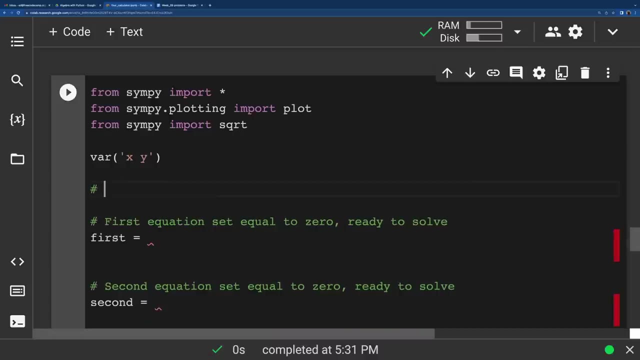 So if we go to our solving graph- and again you might have this and you might have your table of contents, jump right to it. solving graph- We'll call the variables x and y, And you could even write some more stuff in here and, you know, delete it later. So let's take a look at this. 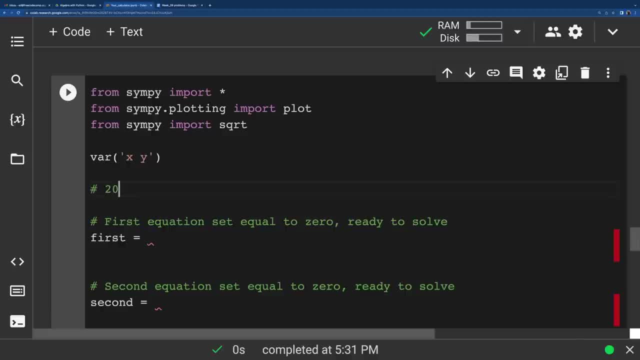 If our two equations are $20 times x- number of tickets- plus $10 times y, how many of those tickets did we sell? equals that total 71,000, let's make sure we get it exact- 71,750.. So now we have an equation for the revenue $20 times this many tickets- the good tickets. 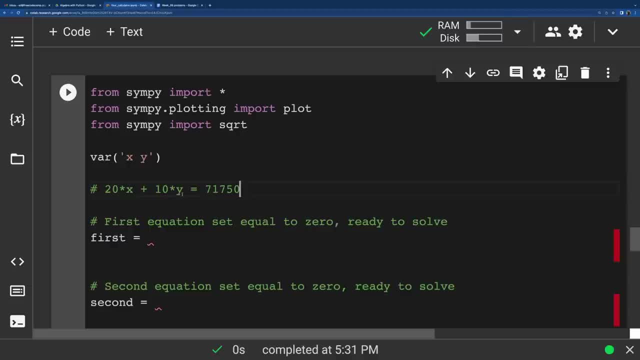 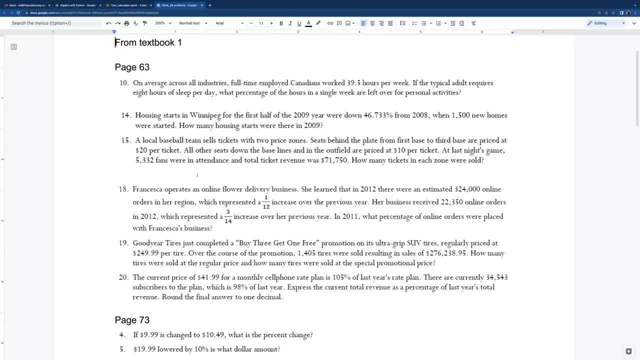 plus $10 times this many tickets that are further out equals this much money that they earned. Now I have two variables. I want to solve this. I need another equation, So what about that second equation? 5,332 fans were in. 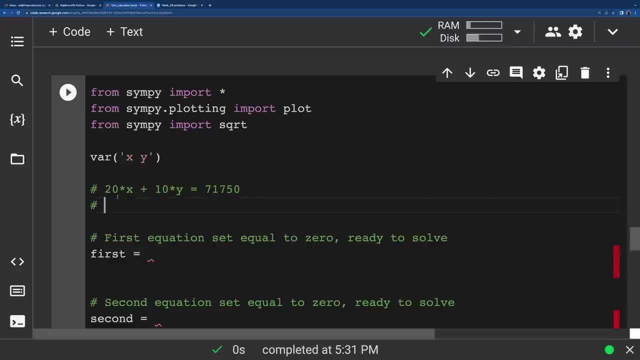 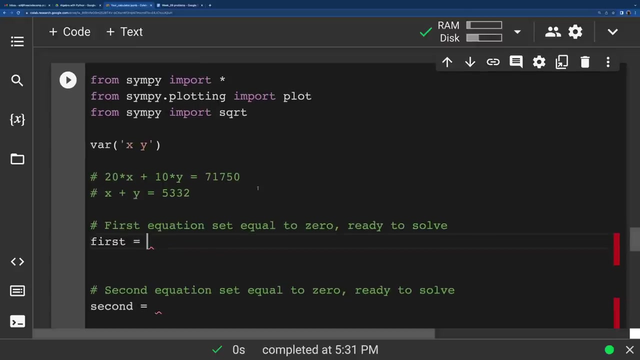 attendance. So x and y were the number of tickets in each section. So x plus y must equal 5,332.. Okay, So in the way we have this set up here, we can just set this equal to zero. So let's take the first equation and we're just going to put this: 20 times x plus 10 times y, and then equal to zero. 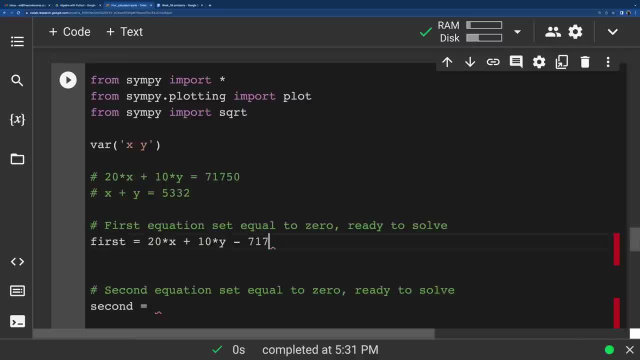 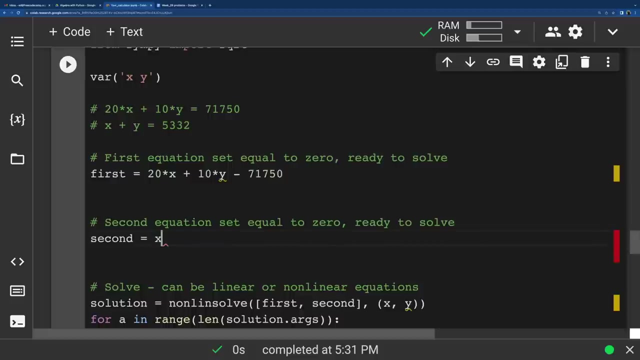 I'd just subtract that other value, 71750, and then that would be that equal to zero. All right, and the second equation: set equal to zero, so x plus y. so I'll do x plus y and then minus 5332, that would make that set equal to zero. 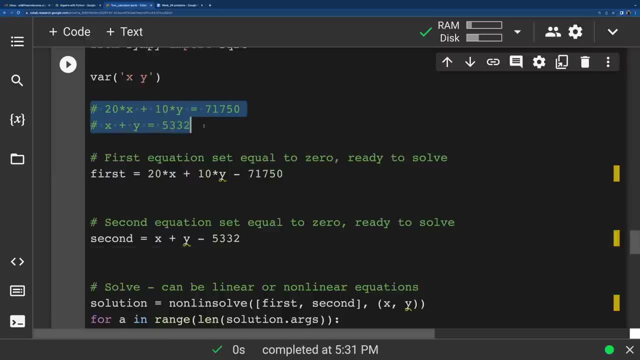 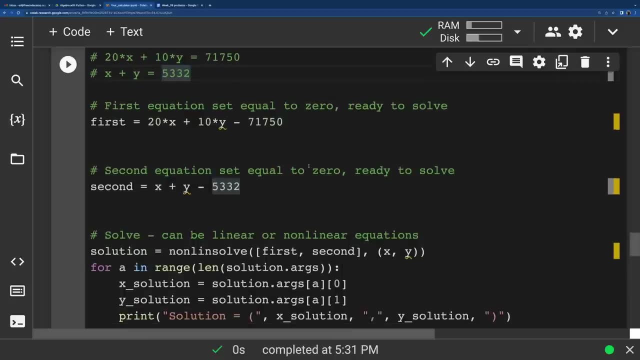 And this is the idea. you can add other things here if you want to factor, and then just setting up these Equal to zero is the easiest way to set up Because, remember, we already set this up to solve, factor it and then graph it. 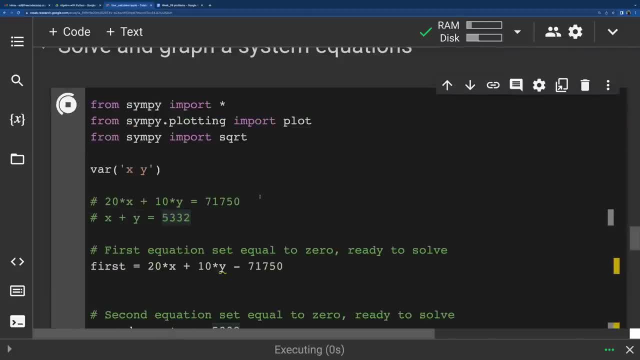 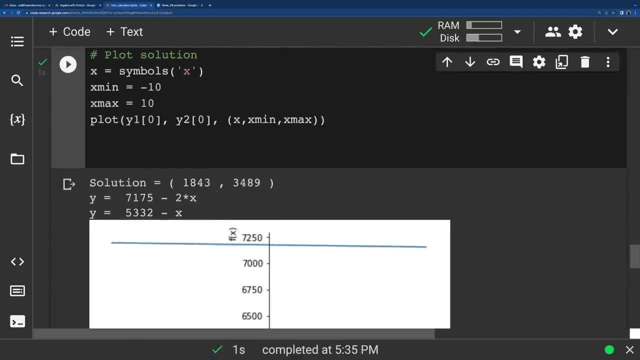 And the graph, you know, just might help visualize it. And when we solve this. so there we go. See the solution here. and 1843 and 3489.. So that's how many Of each, Because when we add these up then that's going to be 5332.. 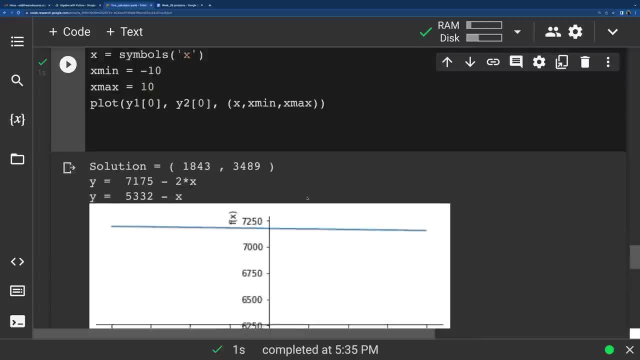 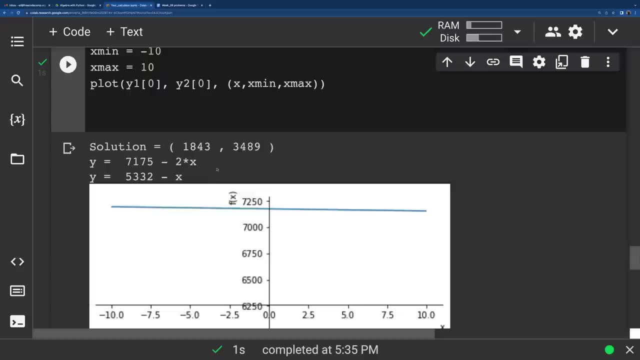 And There we go. Now we know how many of each ticket. So 1843 people Set, you know, From first base to third And 3489.. As we expect, there's more room out there in the outfield and beyond. 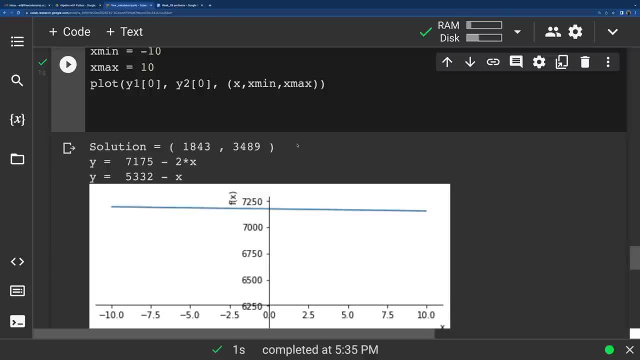 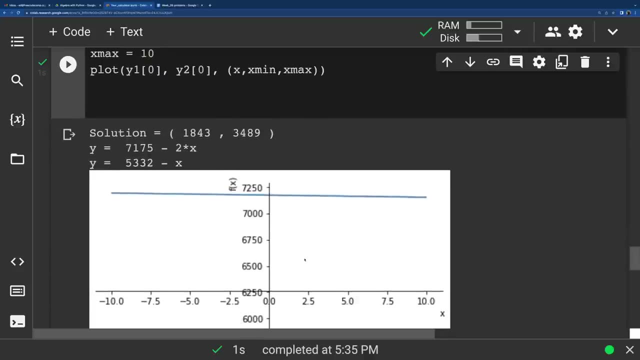 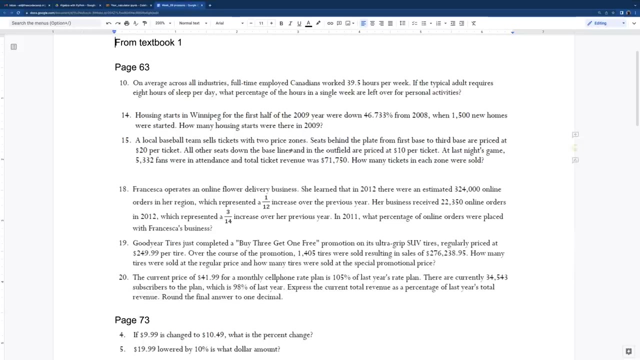 So you know, that's how many people sat out there. And now And now we can figure this out And we see the graph, just to see the comparison here. So pretty cool, We can, we can figure out, given this information, how many people sat in each place. 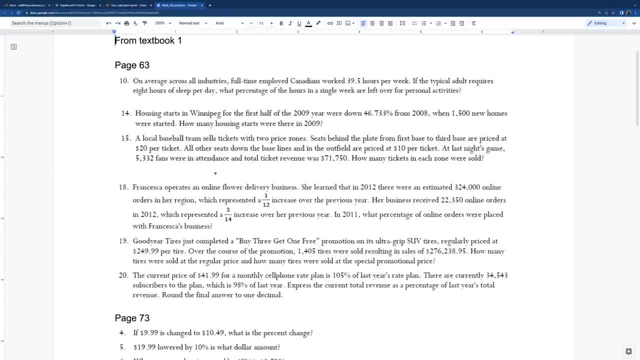 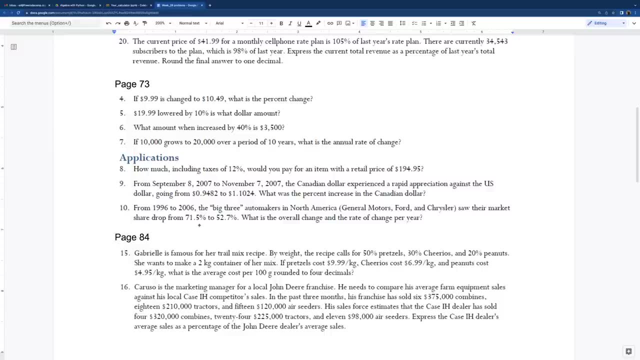 And who knows, maybe if it wasn't totally sold out we can get a, a breakdown All right, And You know some other applications We'll we'll skip some of the percent increase. Maybe we'll take a look at. 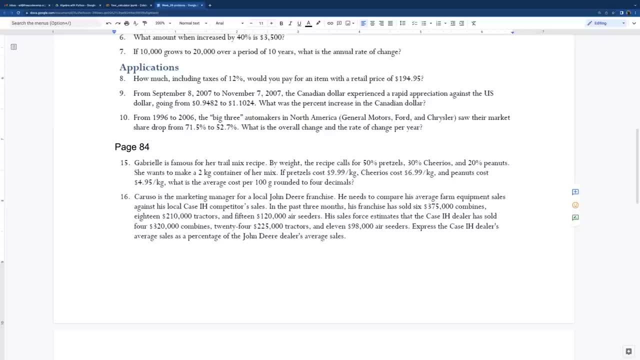 This one here, So number 15 from page 84.. So if Gabrielle is famous for her trail mix recipe, Um, let's talk about the by weight. Her recipe calls for 50% pretzels, 30% Cheerios, 20% peanuts. 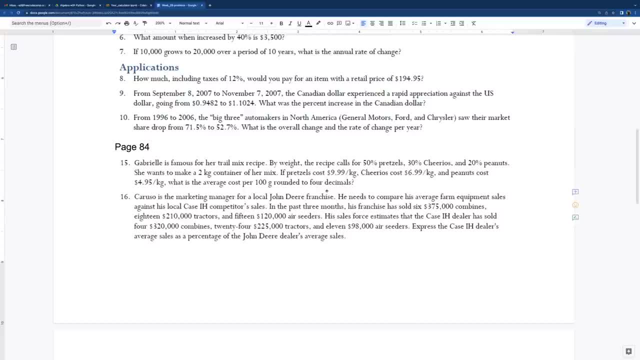 And she wants to make two kilograms Of this mix. So we could just calculate how much of each Of each She's mixing. So pretzels, Cheerios and peanuts, And this one, We could just go right to, right to here. 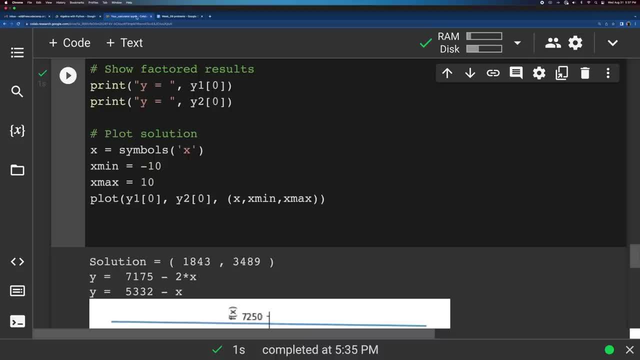 And Before I even get to a print statement, We can just define some variables. Um, In Python we like to use the underscore, So maybe, Uh well, Pretzel Wait, Uh, Uh, no, Uh Uh. 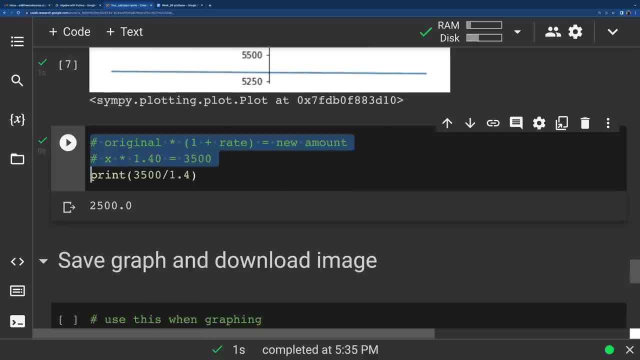 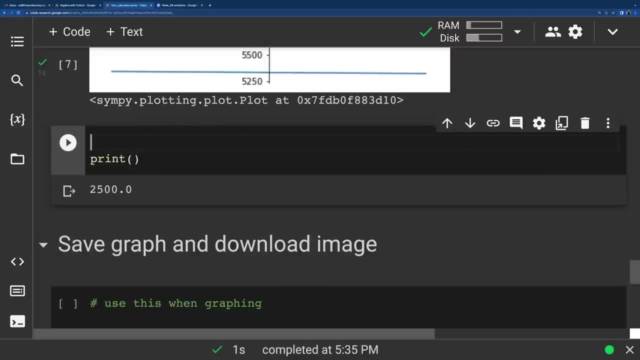 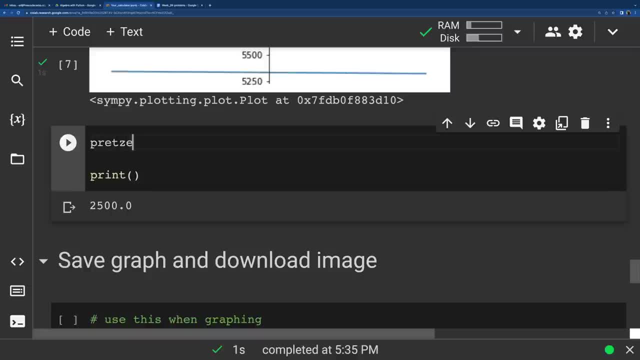 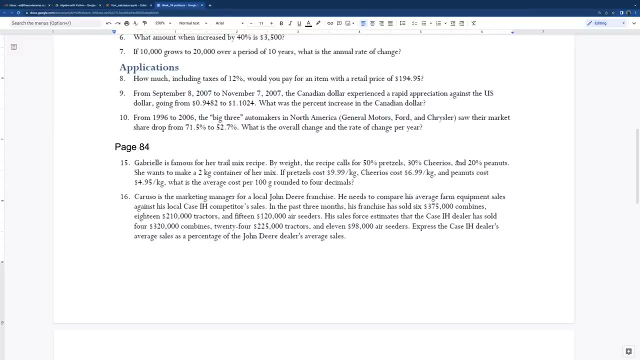 So maybe pretzel weight, maybe we'll do pretzel pretzel there we go. equals 0.5 times 2, because it was 50% pretzels and she wants to make 2 kilograms. Cheerios is going to be 30% and peanuts 20%. 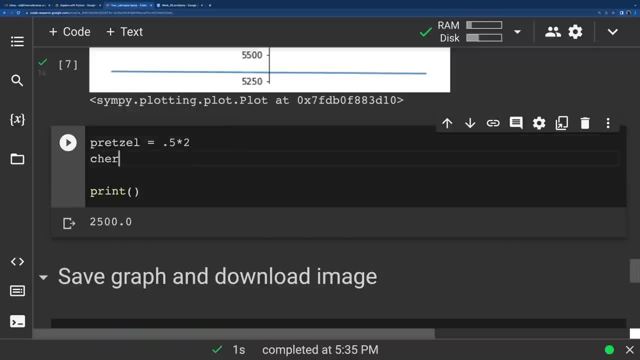 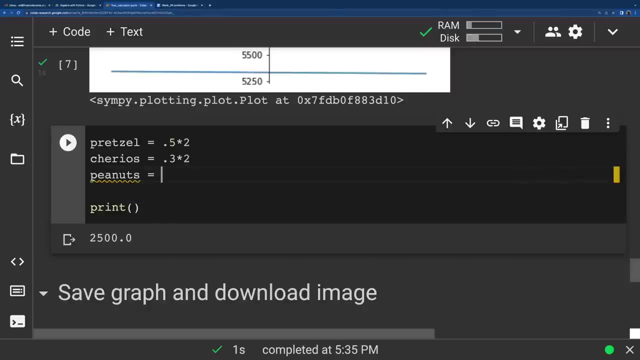 So Cheerios equals 0.3 times 2, and then peanuts equals 0.2 times 2.. Now we know that we have the weight of each of these and you can put comments in there for yourself if you need to. 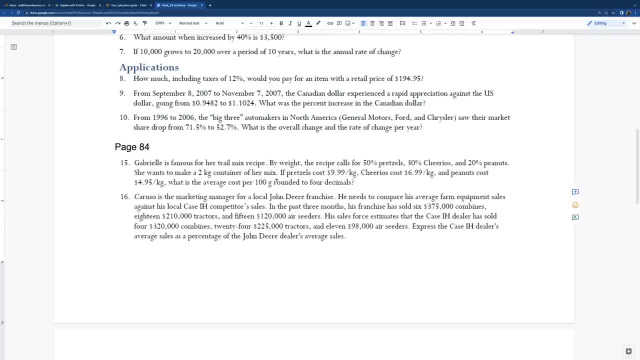 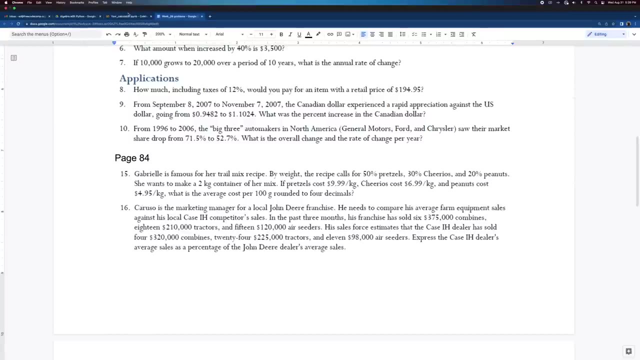 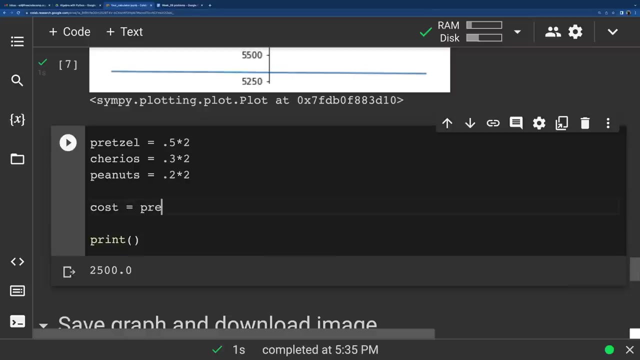 And now we want to talk about the cost. So there we go. So if we have the cost, so all of this pretzels times 9.999.. And so if we have this, our cost equals pretzel times 9.999. 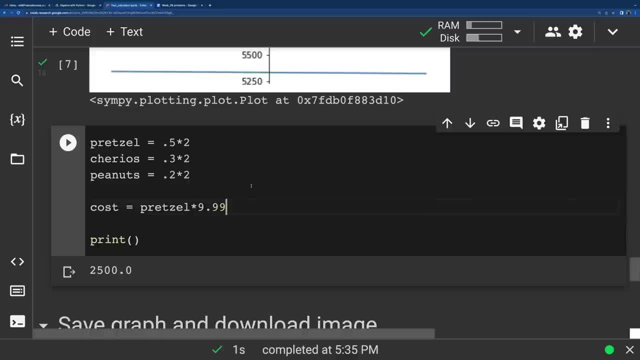 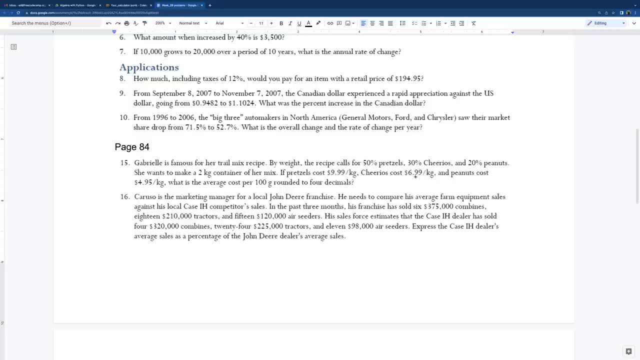 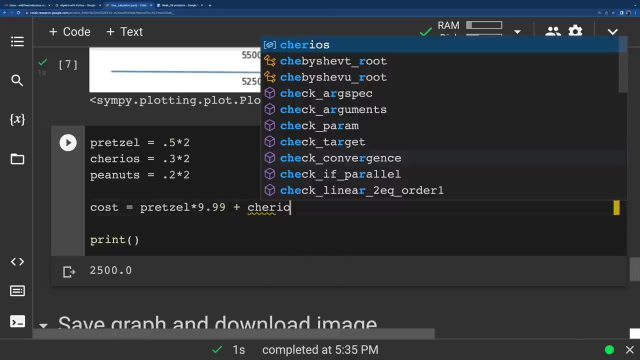 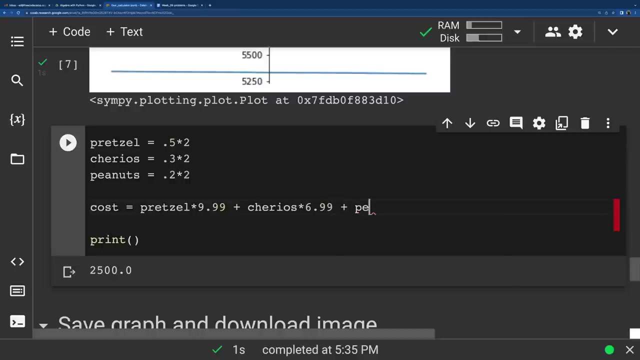 Because that's how many kilograms? at 9.99, a kilogram Plus. and we'll look at Cheerios 6.99 and peanuts 4.95.. Plus Cheerios: times 6.99.. Plus peanuts times 4.95.. 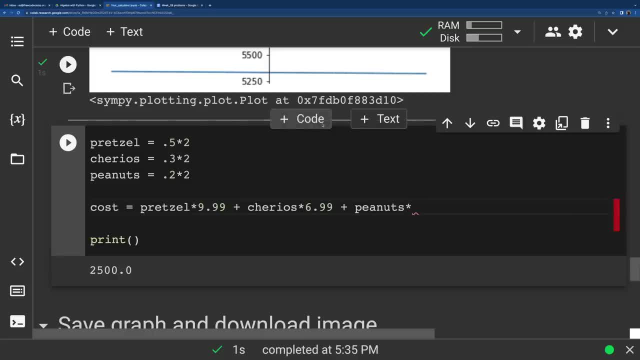 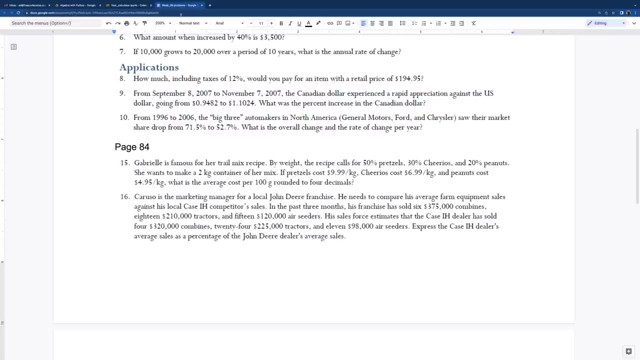 Plus peanuts times 4.95.. Plus Cheerios times 6.99.. Plus peanuts times 4.95.. So now we have the total cost here, and that should be then the cost for 2 kilograms. Fine, 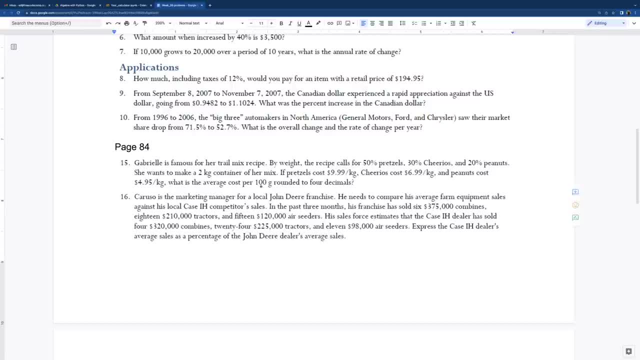 But the question then asks: what's the average cost per 100 grams? So 100 grams compared to 2 kilograms is, you know, a lot of money. So the average cost for 200 grams is divided by 20.. 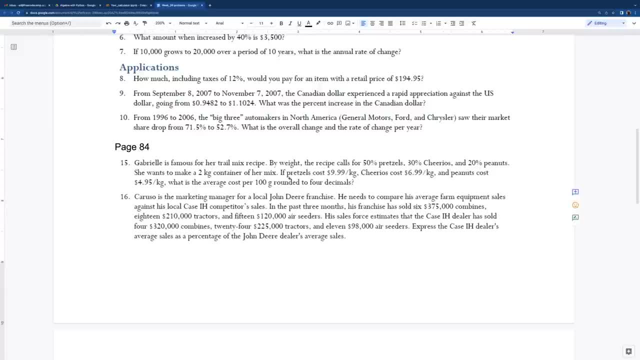 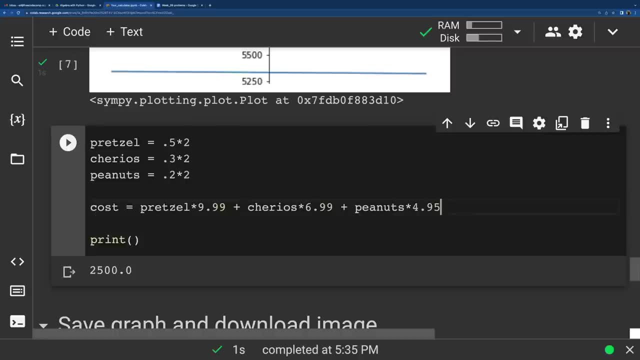 And we could do the comparison if we wanted to also bring it up to the proportion earlier on in this notebook. But knowing that this is 2 kilograms, 100 grams, And so it's, we can just put this in the print statement. 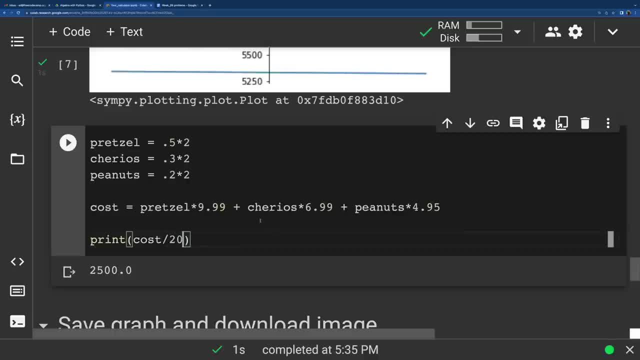 Cost divided by 20.. Because that's the cost for 100 grams. There we go. So how many of each if we're making two kilograms? but then the final question: uh, we need to divide it by 20. we only want 100 grams, and there we go 80 cents, which makes sense, because if we take a 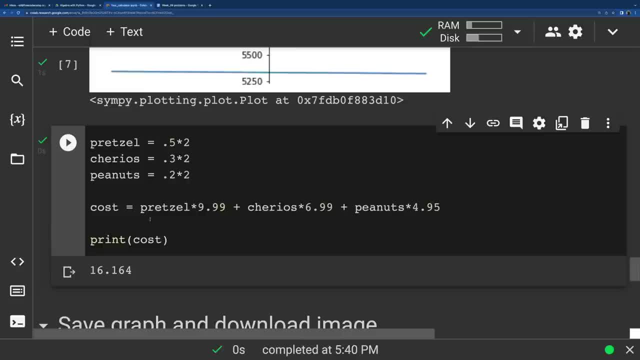 look at the total cost for each of these, yeah, when we're buying the full two kilograms, you know, given these rates, yeah, that's 16 worth the trail mix. i mean, you know, hopefully two kilograms of this, this mix, it'll last a while. so she just wants to make 100, 100 grams. so that's why she. 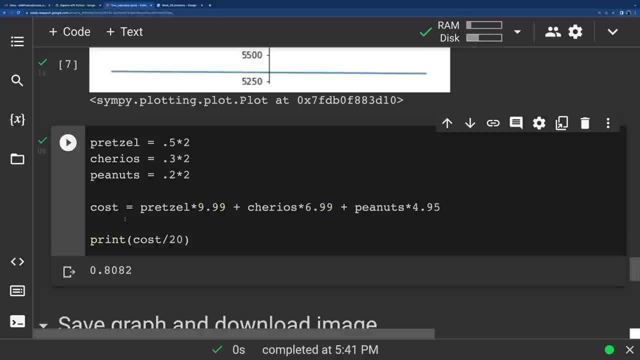 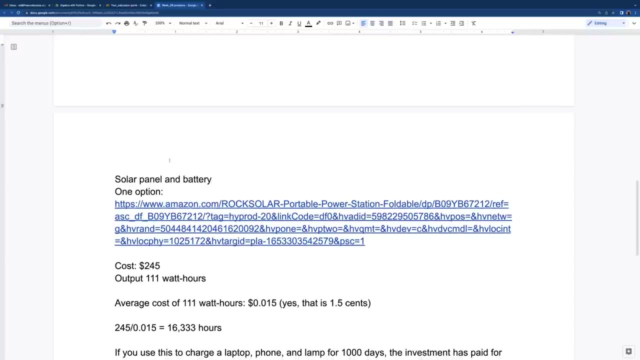 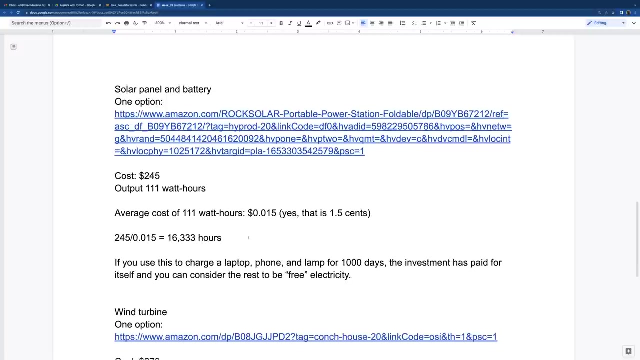 is just dividing it by 20, 100 grams, you know, so that people can eat it before it goes stale. there you go 80 cents. all right, not bad. so some other things that we can look at. making use of these calculators that we have, we can take a look at things like um various like options for things like green energy. 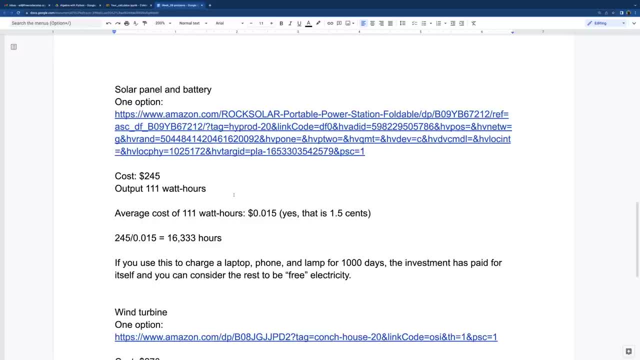 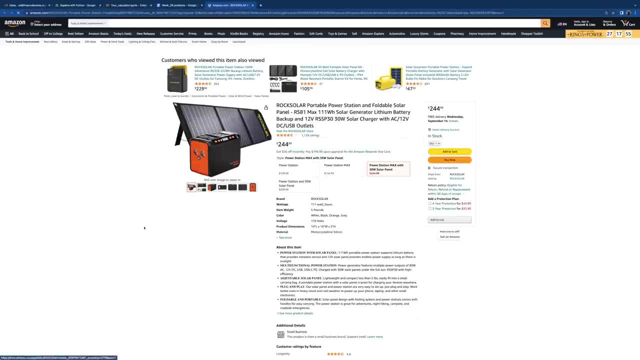 and so i i put in here, you know, just a link to one thing. you know one thing, and it was, i think i did one solar panel, one battery. so supposing you know you want to buy this, you know um, live, live off the grid, or you know. 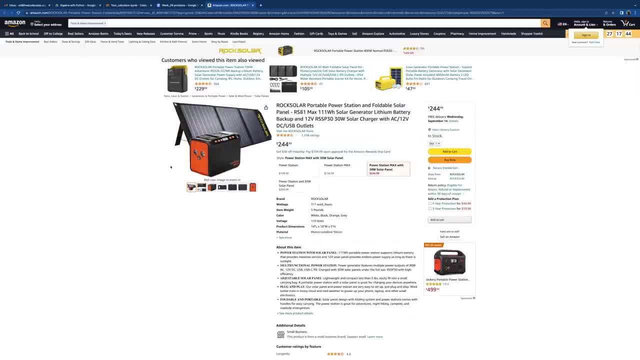 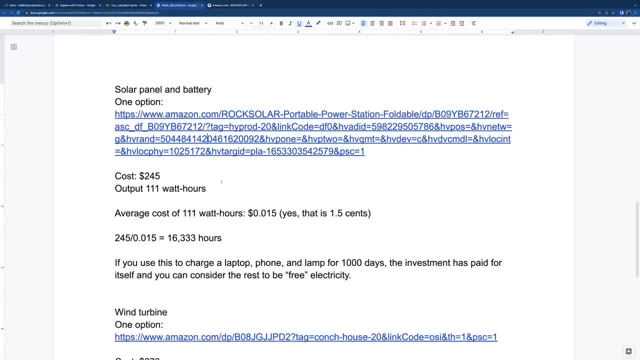 supplementing electricity for somewhere. so here's a solar panel charges up a battery and the cost was 245 dollars, and then the output is 110 watt hours, now 111, so you can certainly recharge this as as as much as possible. um, that's just. you know that output, um, i normally would then think about this as using 111. 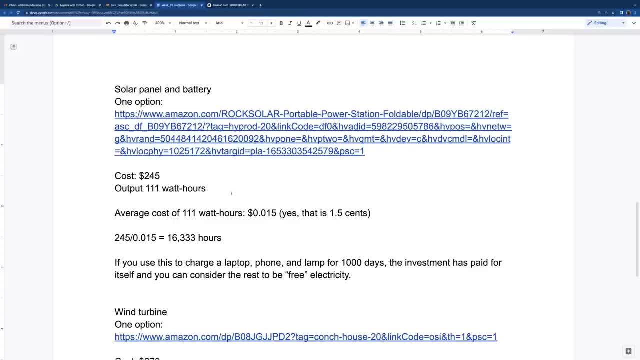 watts for an hour and 111 watts. that should be enough to charge. you know, power your laptop. charge a phone um few light bulbs also. so you know that's something you know you could easily make use of 111 watts. like i said, laptop charge a phone power a few light bulbs, that'll be plenty, and then that way. 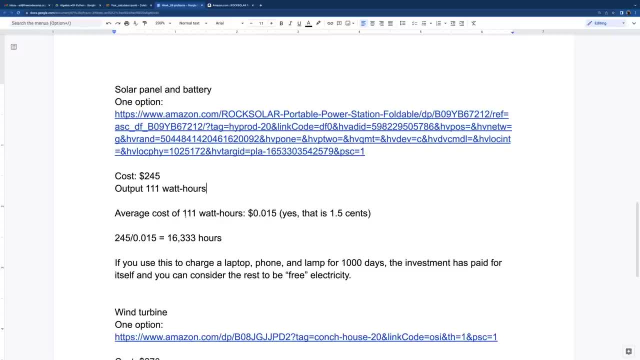 so what? what this would be is so, um the uh, electricity very often is in kilowatt hours, because we use so much and that's like 15 cents, i think, is about the national average. so 111 watts, that's, you know, 10 of that, or a little bit less. 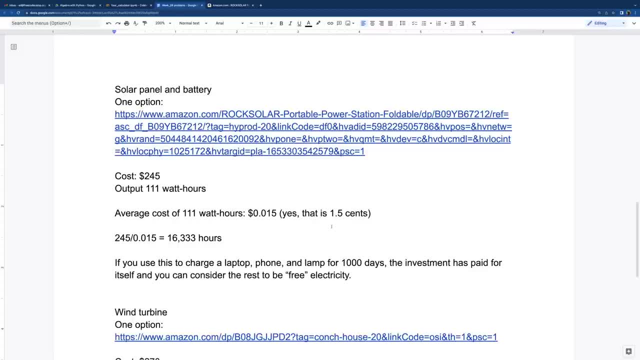 so, yes, that is 1.5 cents. so you know there's 111 watt hours and i was thinking: you know, use 111 watts for an hour, so that would save you a 1.5 cents. okay, now, beyond the savings, if you're also doing this for the sake of being off the grid, or you know. 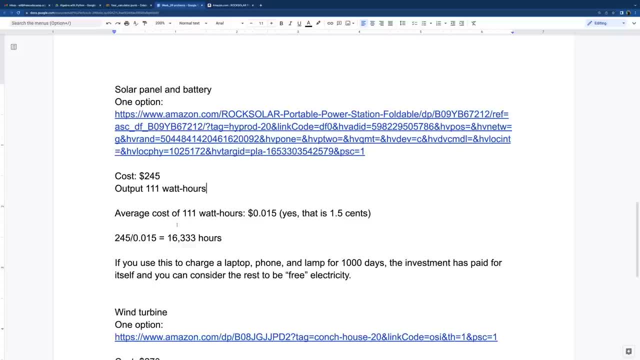 uh, you want to run, run some stuff like out in the middle of nowhere where you can't really plug it in. well, that that's the value of this. but let's just say you want to compare this to electricity cost. so you know that 245 dollars. and if you run this for you know all you're making full use of. 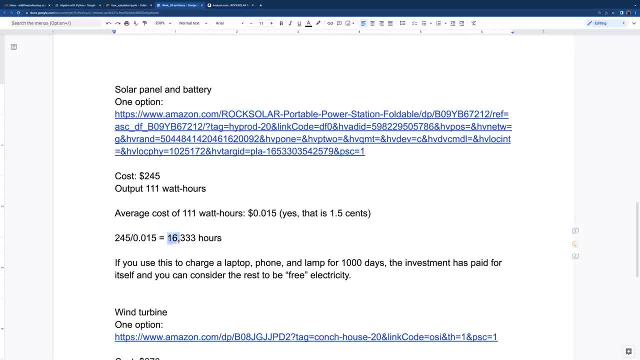 all of this, for you know you're making full use of all of this. for you know all of this, for you know, an hour, then it'd be 16 000 hours and dividing that out, um rough estimate, you know we're doing a little bit of rounding here. thousand days, you know, which is. you know a little bit less than. 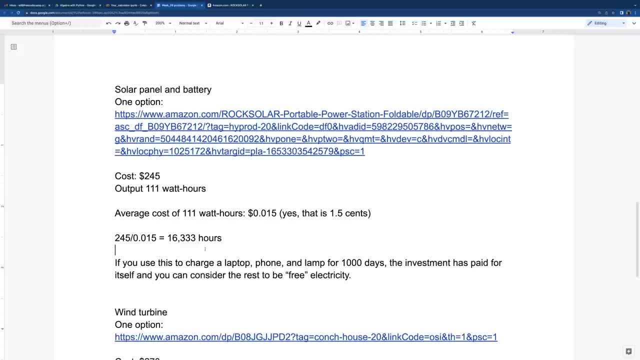 three years, and if you do that you could, uh, you know, pay for itself in a thousand days, which for a lot of investments, that's not that bad. and then, after that, free electricity. you know you paid for this, and all along the way, you know you're. 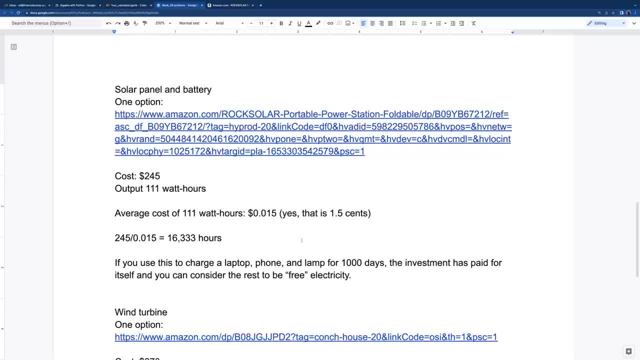 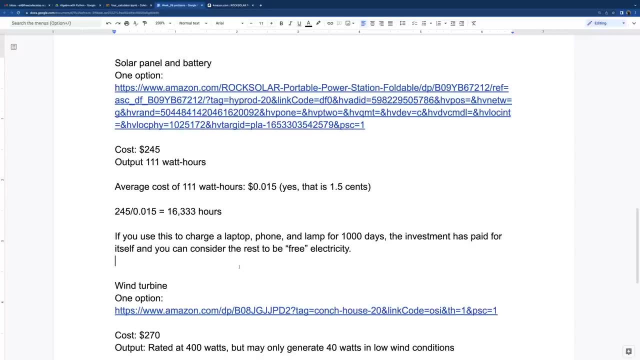 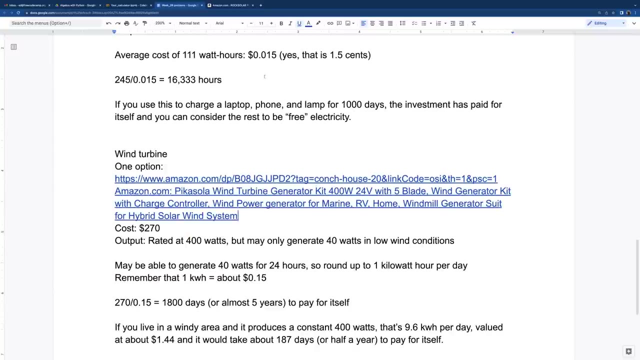 you're saving this money for the thousand thousand days, and then, after that, there you go, you've already saved enough money to pay for it and you get the free electricity. i did another one just as another comparison. so this wind turbine- um, i find all these nice, you know, it's kind of interesting. so 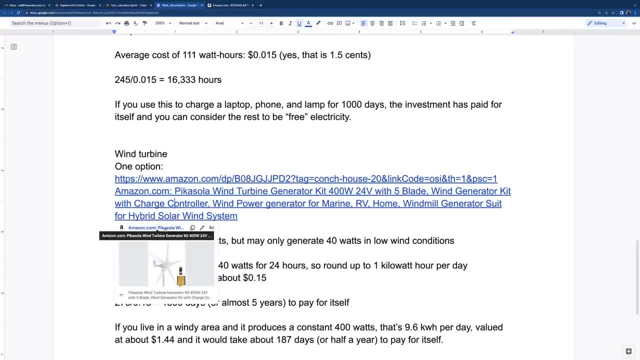 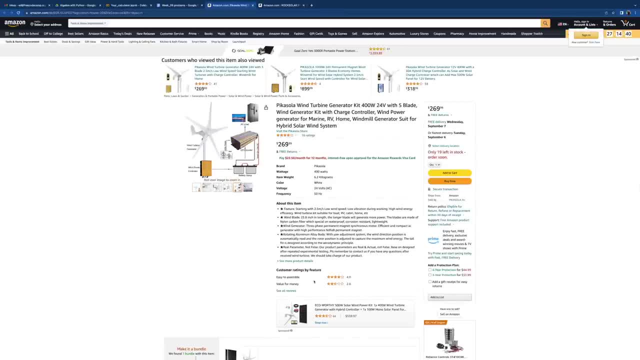 um, did that? i'm gonna go ahead and do that. click, there we go. so this particular wind turbine that can handle like low winds and it's rated for, you know, 400 watts. but, um, the idea is that if it's low wind it might be a whole lot less. 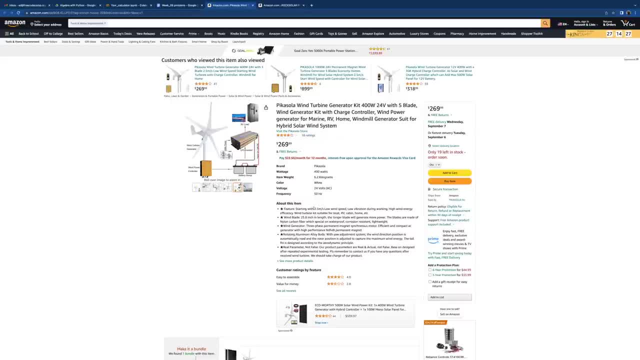 and somewhere in here, you know, it can say 2.5 meters per second, low wind speed, which would be about five miles an hour. and even at that point it'll be about five miles an hour. and it'll be about five miles an hour and it'll turn, it'll generate some electricity. so let's say we have. 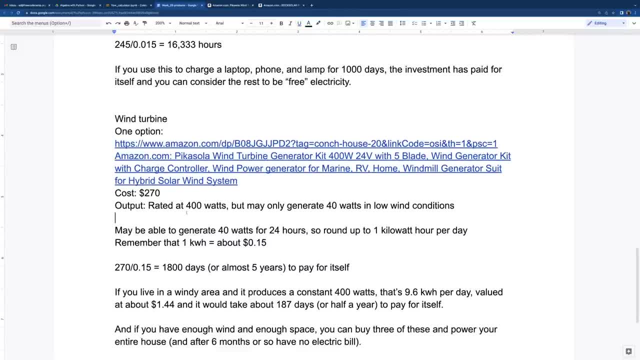 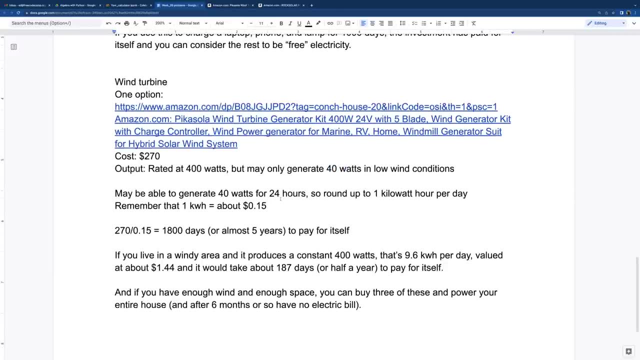 something like this, and this one was 270, 400 watts, but low, low wind, it may just be 40 watts, that's okay. so let's just say you can generate 40 watts for 24 hours because not dependent on the sun, you know you could have wind blowing any time and we round that up to one kilowatt per day. 40 watts. 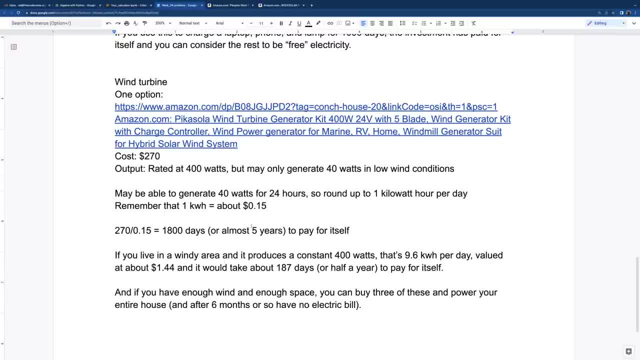 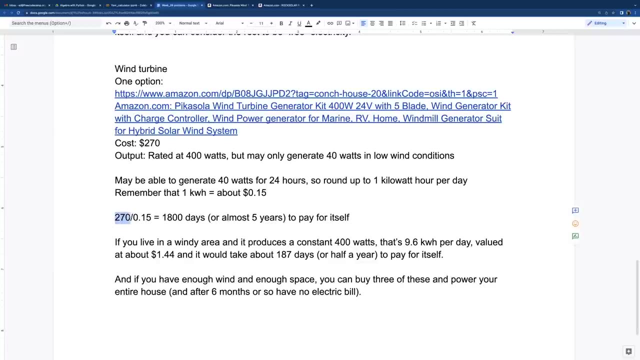 you know, 960 watts. we'll round it up, because this is all just an estimate anyway, so that one kilowatt hour, you know, on average costs about 15 cents. so if you have it somewhere where it's low wind, there we go. that 270 divided by 15 cents gives you how many days- 1800 days. so this one would be if it was low. 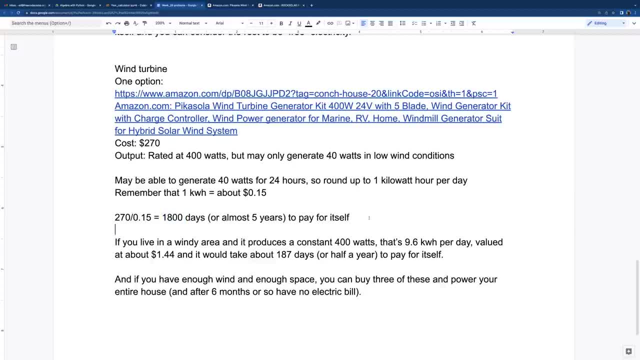 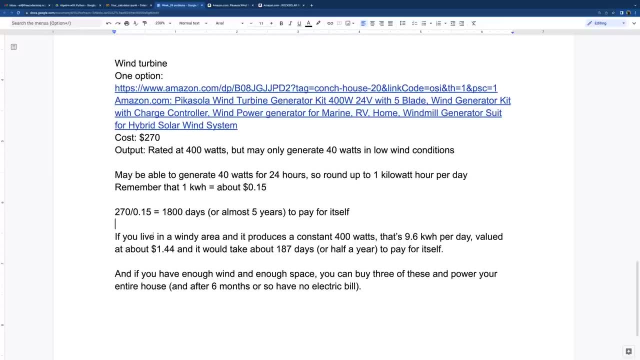 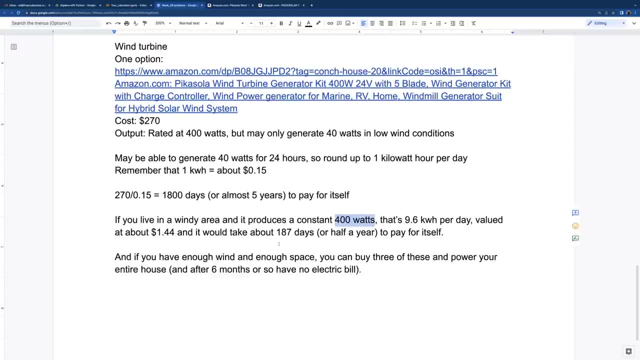 wind. we're talking like five years to pay for itself and then after that you know, free electricity again, even five years, not so bad as a return on your investment. but i just happen to mention if you, if you do live in a windy area and let's say you can produce a constant 400 watts, you know this is. 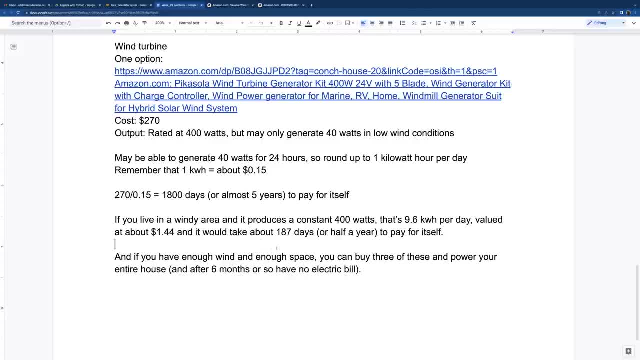 a lot of places you know, especially if you're near, like a body of water, sometimes lakes, ocean bay, you know wide river, you could definitely get a consistent wind. and if that's the case there you could get a consistent wind and it would only take about half a year to pay for itself. because if 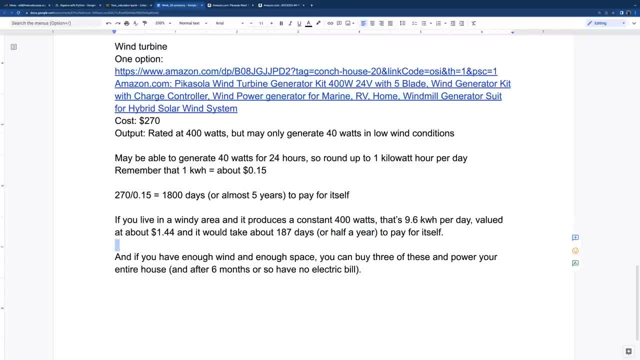 you're producing this 400 watts, that's 9.6 kilowatt hours per day, or $1.44. and then just do that division: you know 270 divided by $1.44, 187 days, you know just over half a year, and really then, 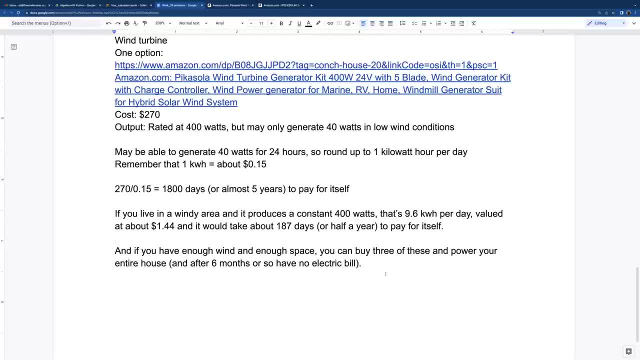 enough wind in enough space by three of them, and because you're making, you're making a lot of money, you're making a lot of money and you're making a lot of money and you're making a lot of money and you know you're generating 400 watts um. three of them is probably enough to power, you know. 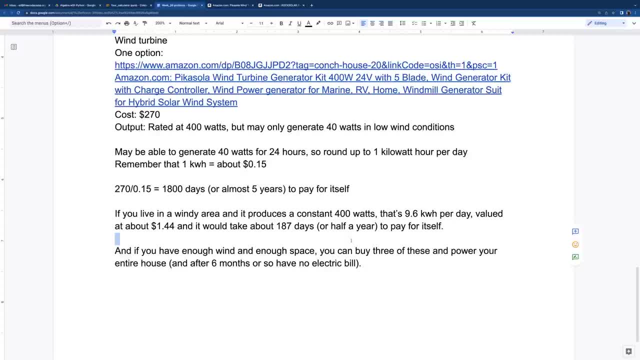 somebody's house like everything. so you know you're. you're saying you would be saving all that electricity, you'd be making use of the three of them and power the whole house in about six months. so, uh, you know the same, that it would be that about that same. yeah, so really interesting. 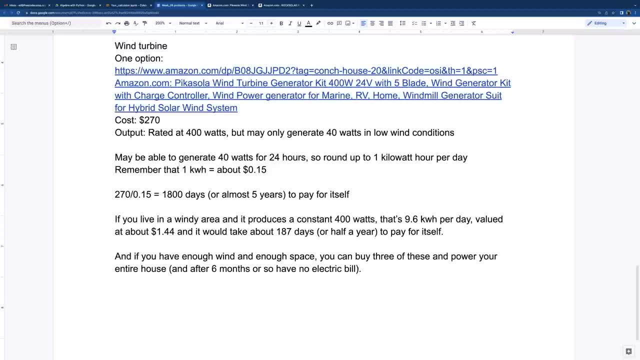 and this is the thing: like you can do these calculations um, i just wrote them here, but you can also bring up the google co-lab and do these different calculations um graph, different things, if you wanted to see, see it, and that that that's the idea with having all all you know, all the math calculations you know, at your fingertips. 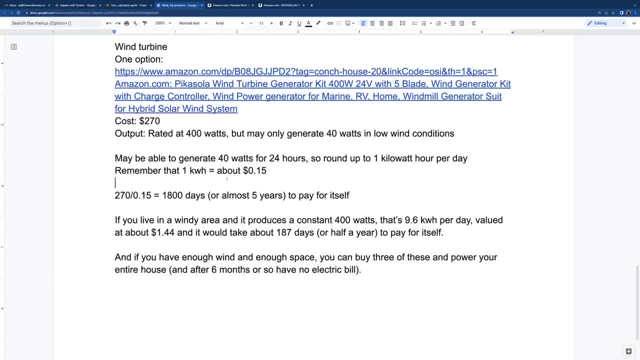 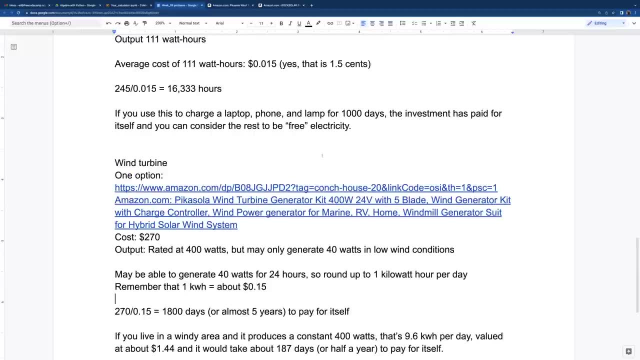 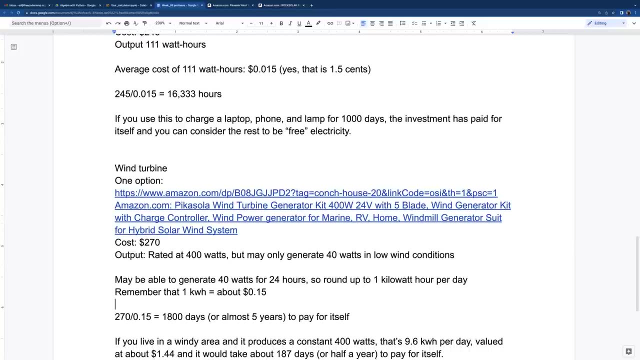 you can count, you can calculate things and figure out: is it worth it for me? oh, hey, if i spend this much money and then, you know, generate this for electricity, yeah, maybe, um, or or you might say: um, it's not a priority right now and you know that's it, but you but. 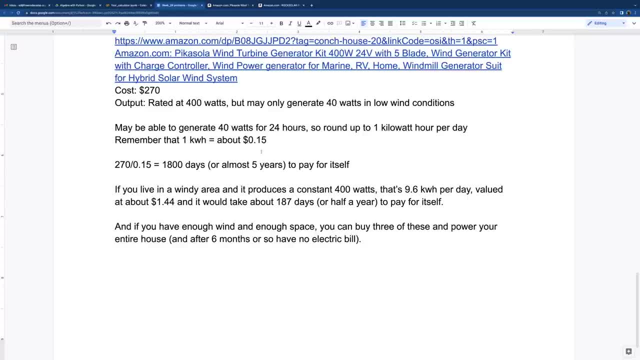 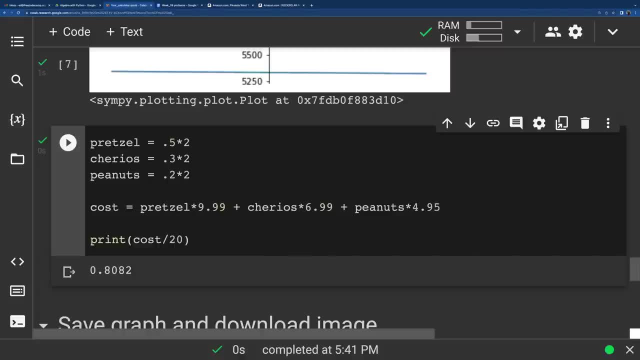 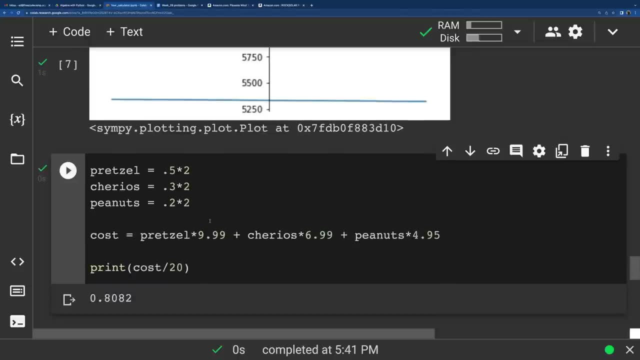 you know, based on the numbers. so that's, that's really some of the, some of the uses of, of some of the math we've been doing and, you know, also making use of, you know, the co-lab of graphing some different things or solving, solving some problems. so hopefully this was. 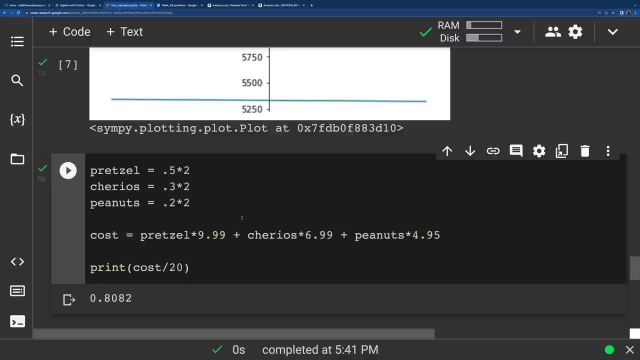 this was useful and hopefully this gives you ideas of other things you can do. once you set up your your uh co-lab notebooks and you have the ability to calculate and graph some different things, um, you know, make use of it to see what you can do to make money or save yourself. 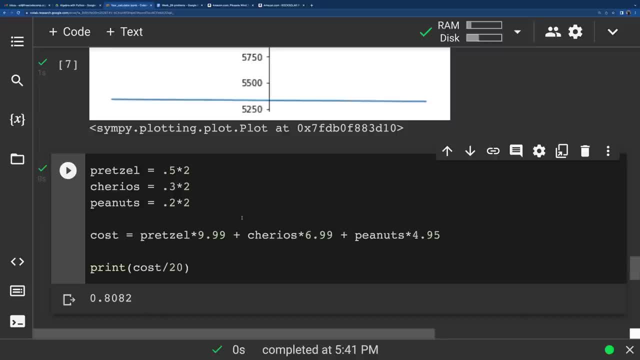 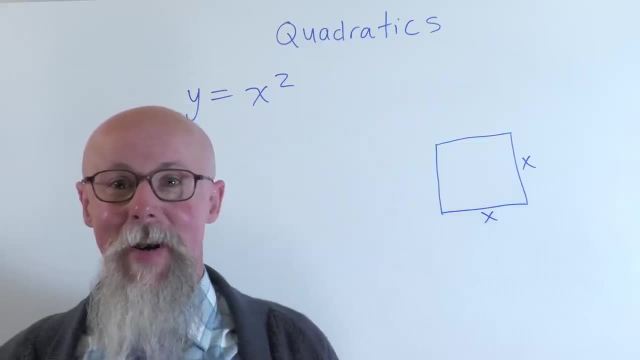 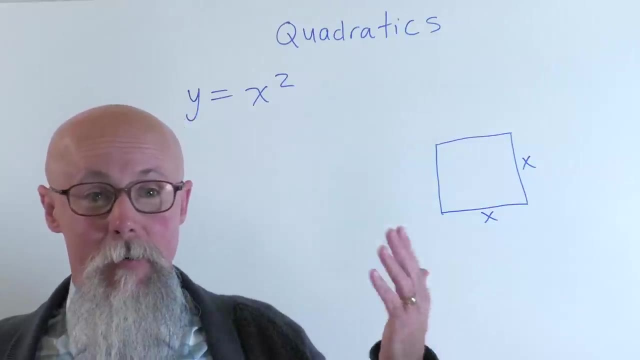 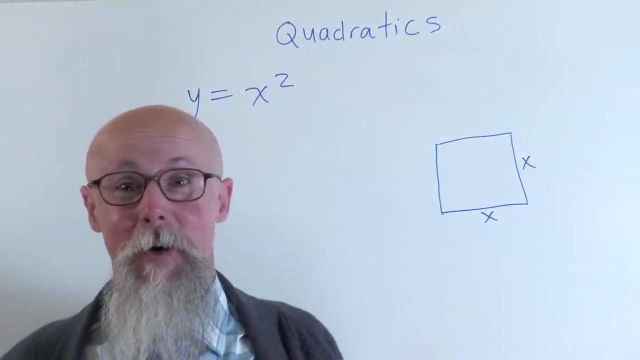 money, all right, and we'll go on to the next unit then. so let's talk about quadratics. so the word quad means square, so why would we have, you know, quad square, but then it's, and we call this x squared, but yet there's a two. so where does the square come from? the square in quadratics comes from the idea and 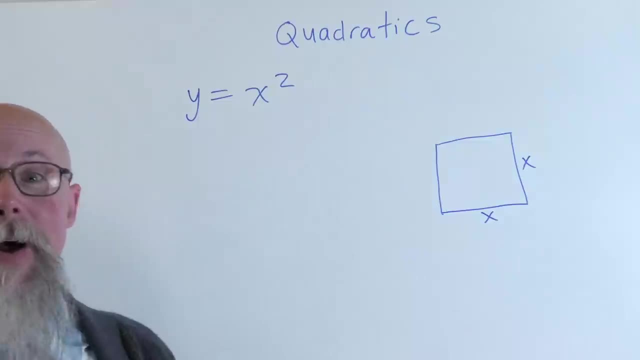 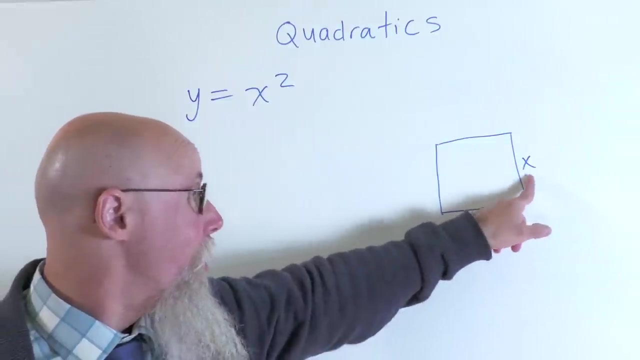 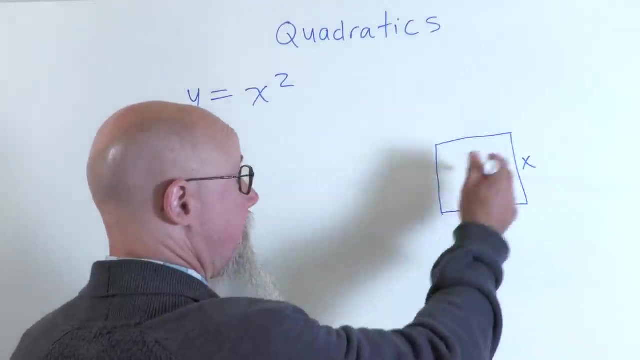 this goes back to the original algebra um, back with al-khorizmi um. so the. if i have a square- and you know, i don't know each side, i'm just going to call them x, but then the area of that square would be x times x, would be x squared, and that's where that's really. 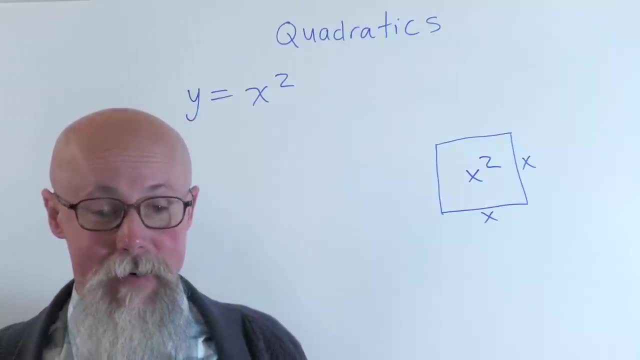 where this notion of quadratics comes from, you know as actually tied to physical area, the area of a square. but there's a lot of other applications and this comes up so often that we get beyond even the, the actual measurements, and we can use this for a lot of other things. so we look at the our. 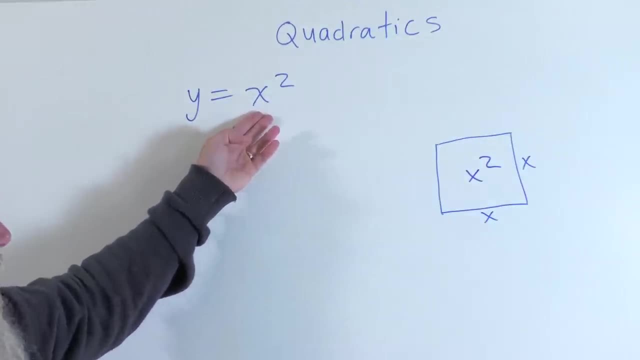 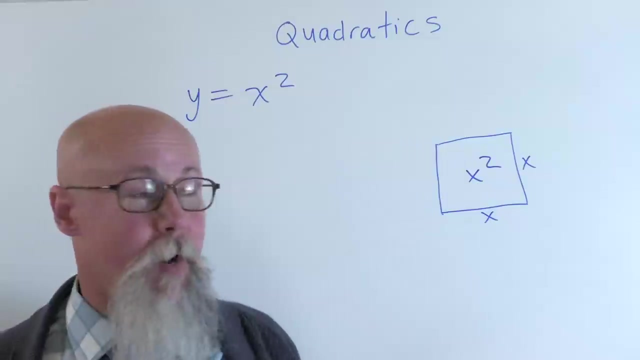 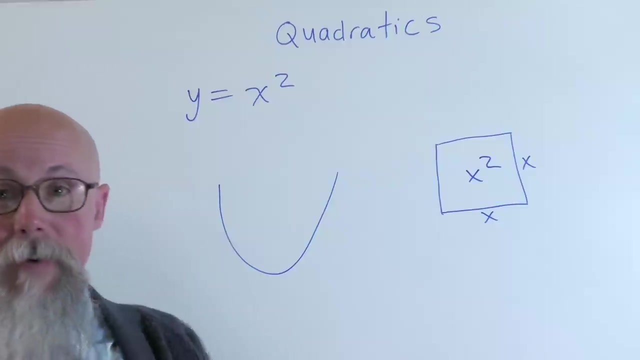 equation: y equals x squared. so if i were to graph this, and when we get into the code, we're going to get into the graphing and we're going to look at some of those applications too, but when i'm, when i graph this, anytime i graph a quadratic, it's going to be a parabola and you know it'll probably look. 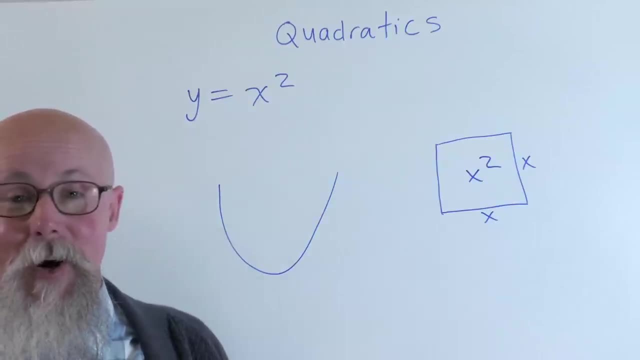 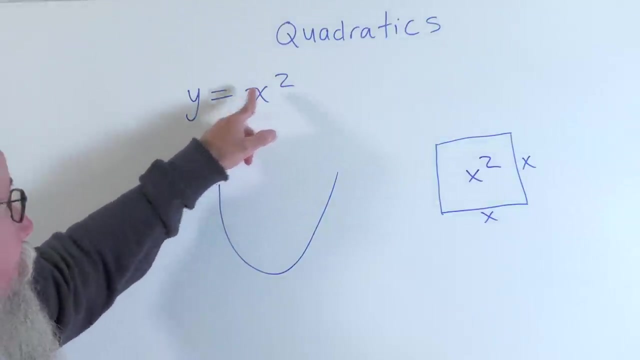 like a nicer parabola than that, but it'll be a parabola. so that means you know, and if we can picture this, the positive values for x give me, you know, i square them and give me some y value, but then the negative values. when i square that, negative times negative makes a positive. 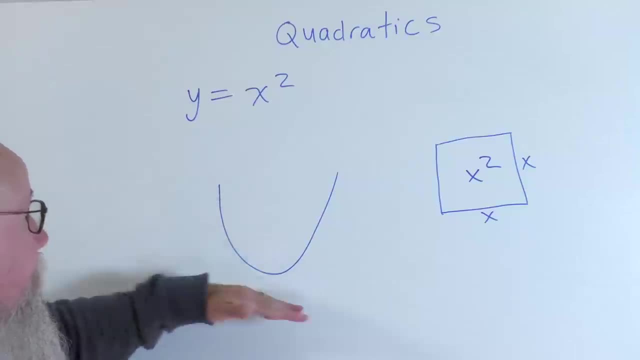 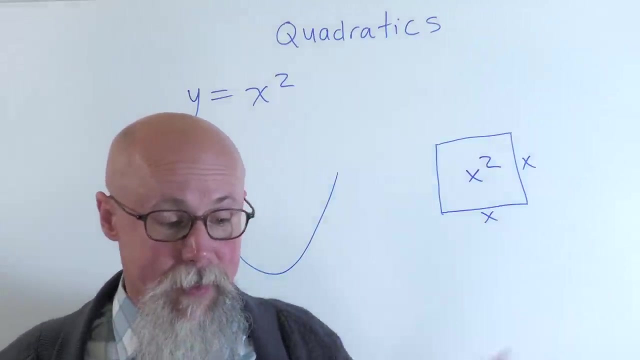 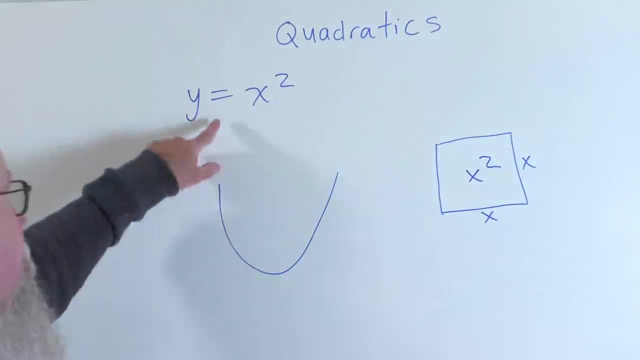 so that's why it curves back around, and so you know, we keep going up and then these two ends go on as long as you want them to. um, but yeah, the the negative x values get squared, so then the y values would still be positive. i still can get negative y values because if in my graph i 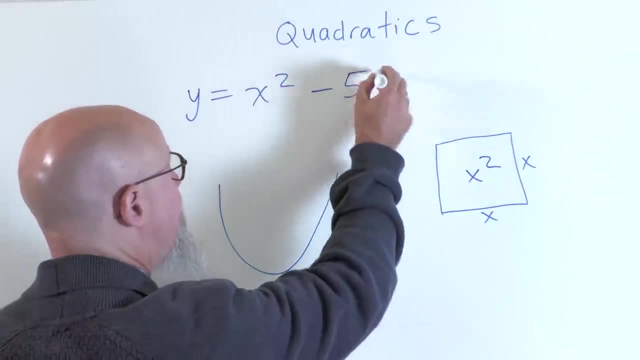 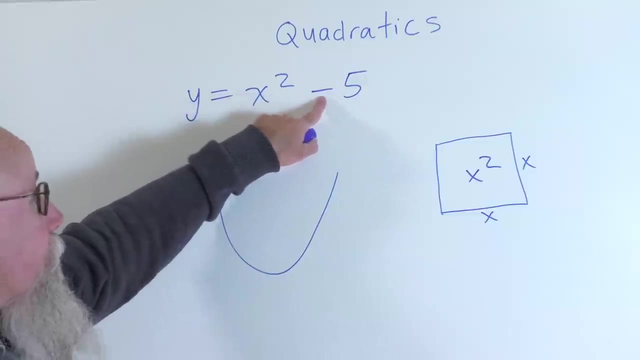 subtract something you know i can subtract. you know five or something like that. so those are. there's definitely some x values there that even squared are less than five. so when i subtract i get a negative y value. so you can still do that, but you see the the general trend of the parabola. 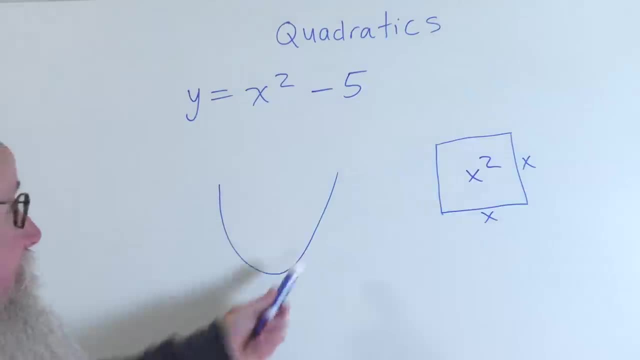 here and they, you know, kind of look like a smile. but if you have, if you have a negative x value, so any negative x value, it looks like a frown. so our code is going to be a negative x value and then we're going to get a negative x value. 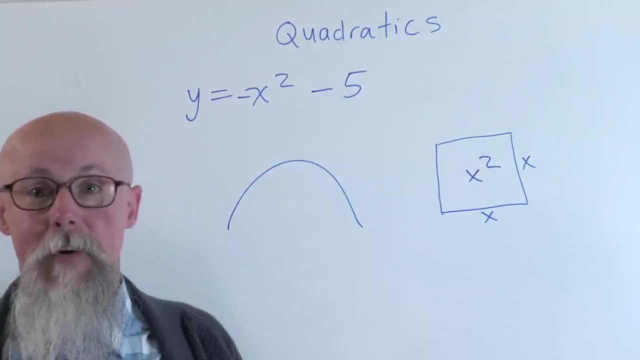 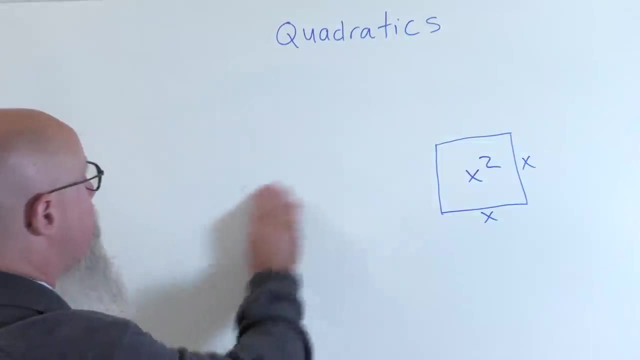 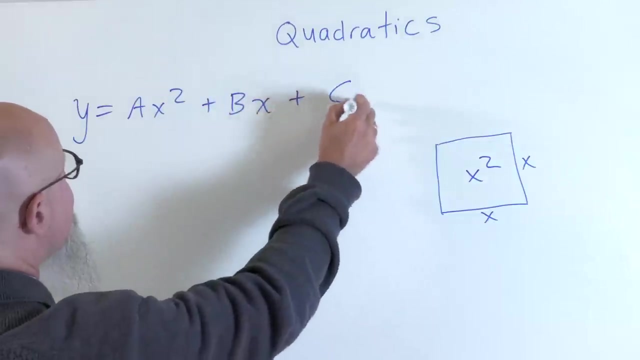 so the coefficients here, um, that one would would be negative. so let's, yeah, let's, take a look at this. if i had any general quadratic- and this is the general form, so if i have, the general form of any quadratic- would be: y equals ax squared plus bx plus c, and that covers all the possible. 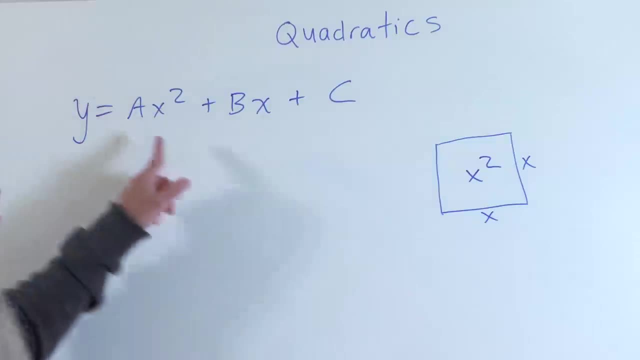 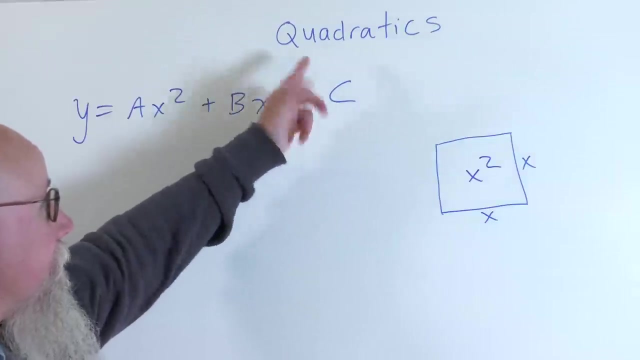 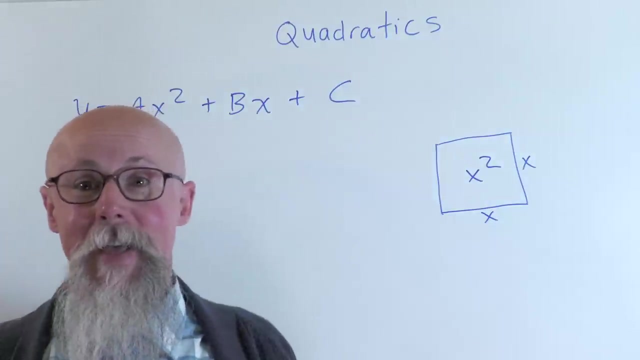 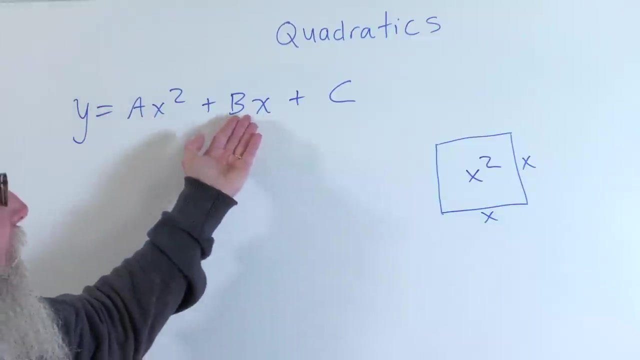 coefficients for any quadratic equation. so a would be my coefficient for the x squared term, b would be my coefficient for the x term and then c would be the constant. and if i look at these, as long as a has a number, then i can have a quadratic b and c can be zero, like the original. y equals x squared. oh well, there's no x term. b is 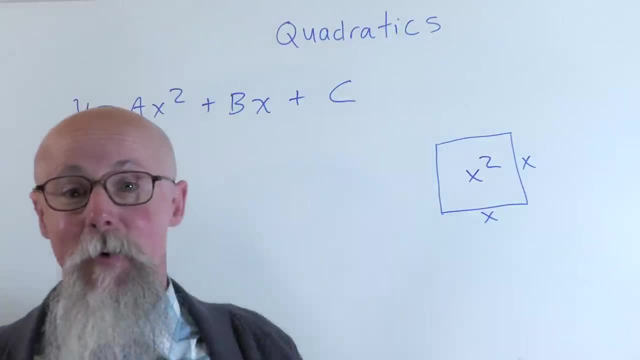 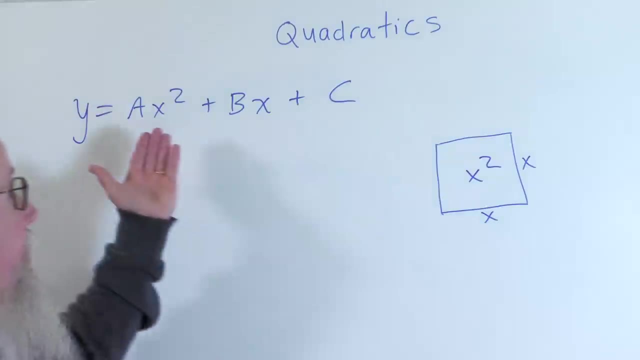 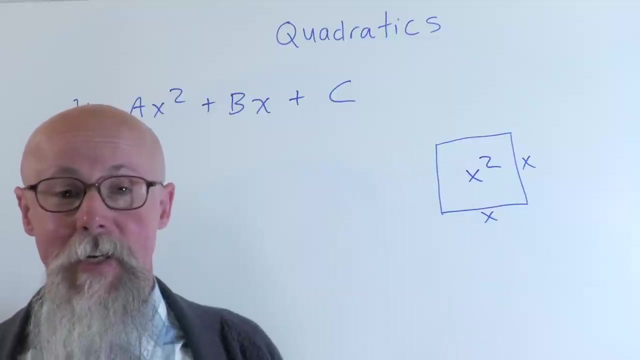 zero. c was zero, um, and then the other one i brought up, i put minus five, so then c would be minus five, zero. so there we go um the general form for any quadratic, and as long as a has a number to it, then it's a quadratic. a just can't be zero, then it's some some other type. so if we take a look at, 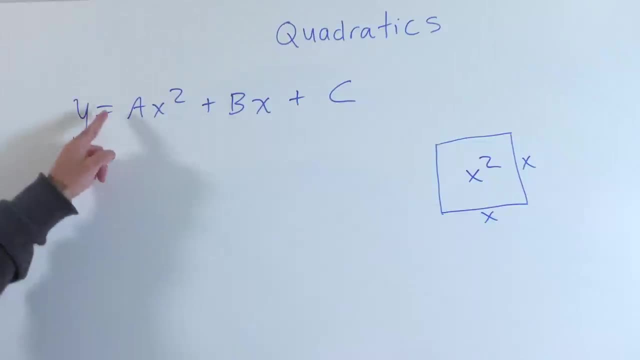 this, and you know, a is negative, it opens down like a frown, a is positive, opens up like a smile. and the other thing about these quadratics is they're all symmetrical, so the vertex is the point at the bottom or at the top, depending on how it turns, uh, of where the 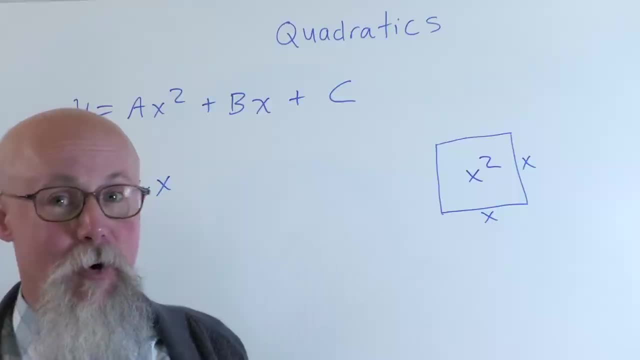 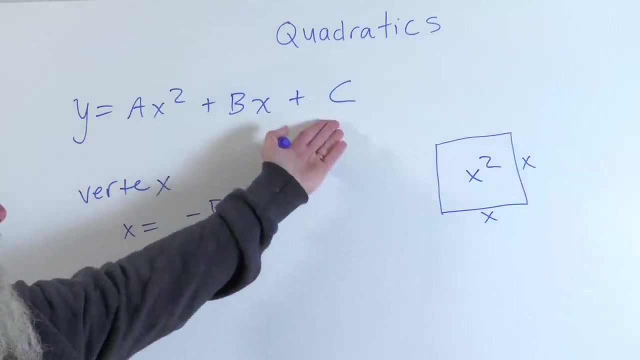 gravel turns around. so since it's symmetrical, the x value is going to be this definite formula: negative b over 2a. so what i have is, once i have a, b and c, i can plug in my four, my values for a and b and get the x value for the vertex, and then, once i get the x value, i would plug that x. 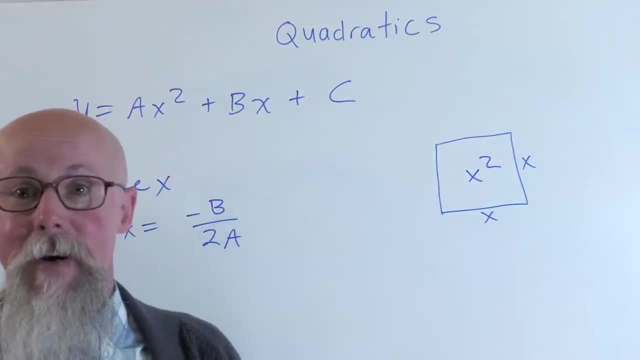 value in to get the y value, and then i'd have this point, and then that would be the point: that if i had my parabola, that would be the point at the very bottom where it turns around, and also just looking at that x value, remember, they're symmetrical, so that would divide the parabola. 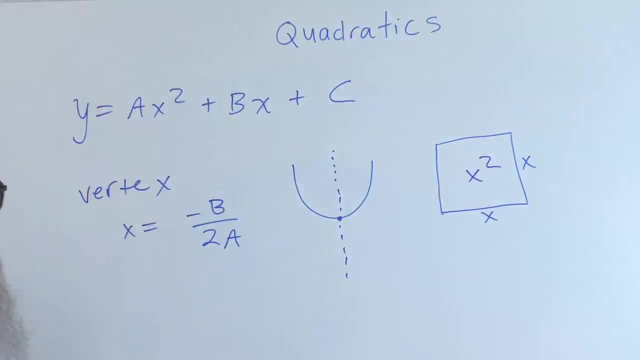 nicely, um. so we're going to look at this, and we're going to look at this, and we're going to look at um doing this in the code, importing a, b and c and then finding the vertex, um finding a lot of other things, so we're going to make use of the code to be able to do that. so i'm not going to. 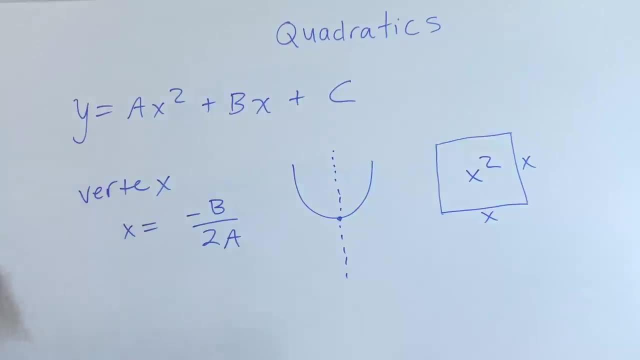 worry about all the factoring here, but what i am going to show you is one other thing, that we're also going to look at the code. but sometimes it helps to see. this formula is a lot of times when i graph this. if i were to graph the parabola, you know, here's my x value and then i'm going to look. 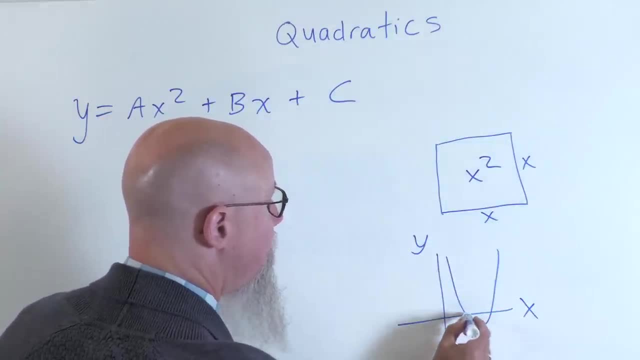 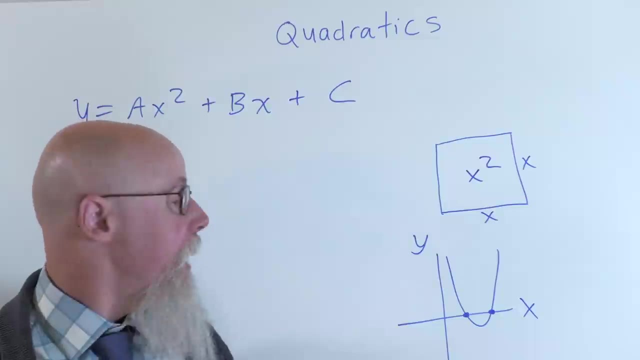 at this y and you know, let's say i have a parabola there. i might also be interested in the roots. where does the parabola cross the x-axis? and so when it crosses the x-axis, then y would be zero because you know, i'm on the axis, i'm not going up or down at all. 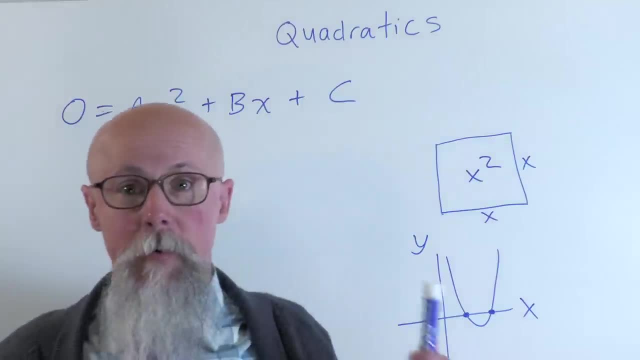 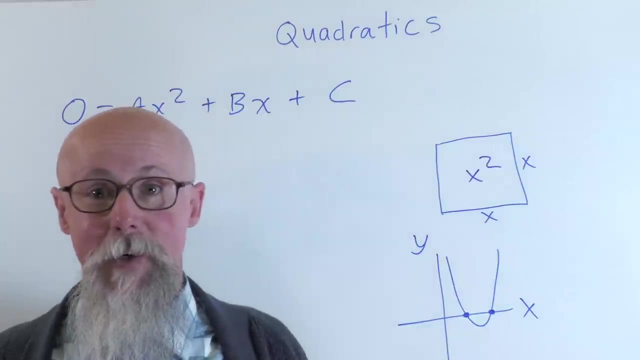 so if i have something you know we would talk about solving for x. but if i have something like this- yes, i have equal zero and i have one variable, which is x, how would i solve it? we approach it a little bit differently than we would the other, the other ones, because when i square root something and that's going to, 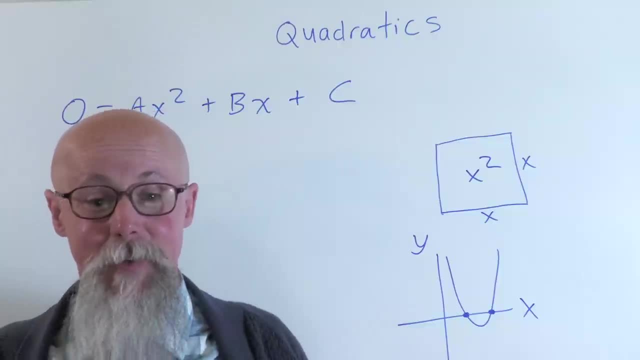 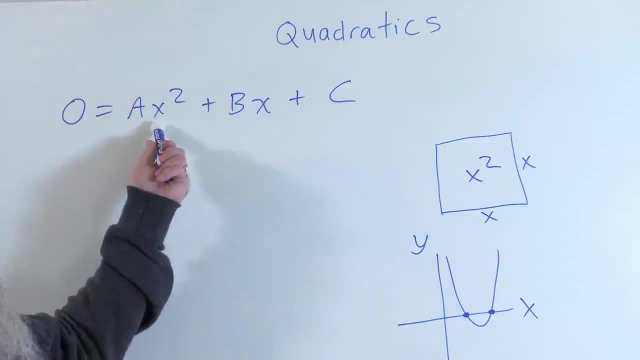 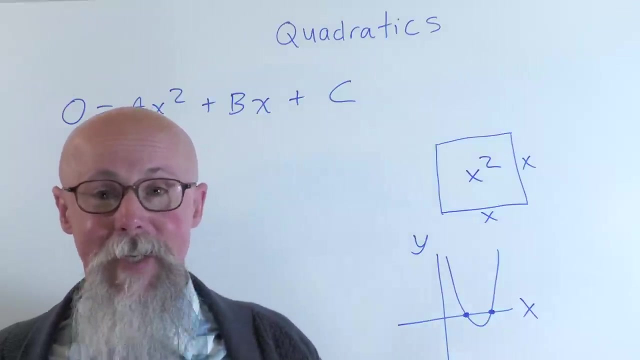 happen as a part of the process. when i square root something, the answer is the positive. there's positive or negative possibilities, because if i had, um, if i had the square, if i had, let's say, four and then the square root, that it's positive four or negative four. 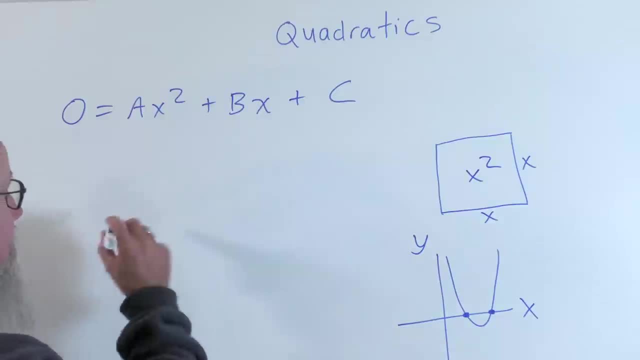 because if i had um positive two, because if i had two squared, that equals four. but if i had negative two squared, that would also equal positive four. so if i'm going the other way, if i have a four and i'm square rooting, yes, it could be positive two, or it could have been. 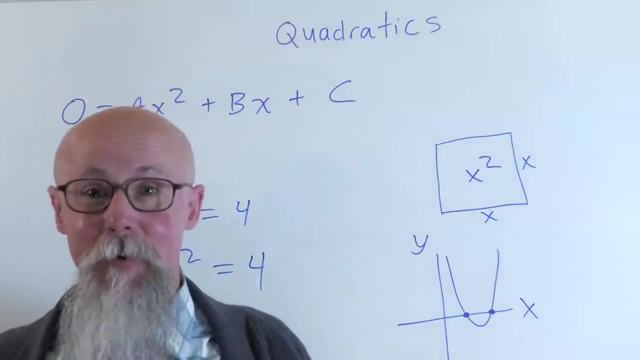 negative two, and so when i'm finding the roots for a quadratic- you know setting this equal to zero- one of the steps is going to be to find the roots for a quadratic, and that's going to be going to involve square rooting, which gives me a possibility of a positive or negative answer. 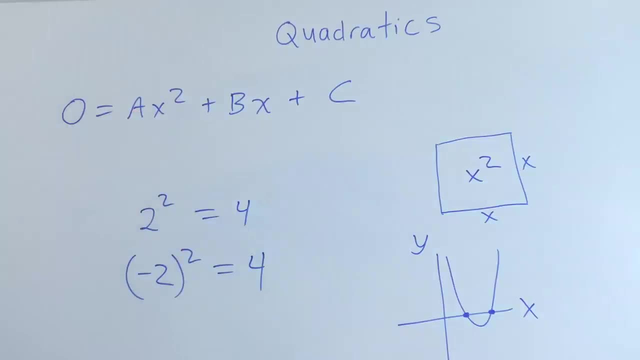 and then that's where we have. you know our two possible answers, and so that's how, in one formula. you know many quadratics, you know the way they cross. they're going to cross the x-axis and touch it twice, so to find the roots. i want to find out those two values and the formula will. 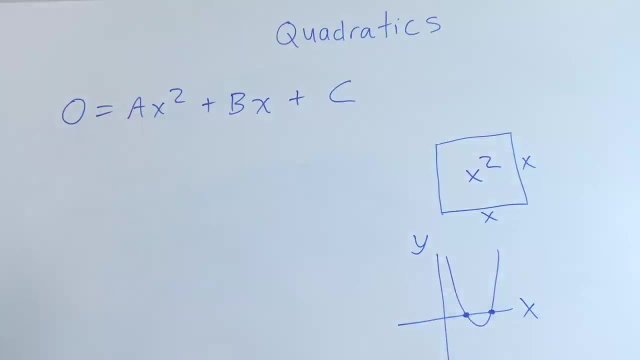 give it to us. so, again, knowing a, b and c, the quadratic formula is going to be a square root of b, squared minus four a, c, all over two a again. so this is the quadratic formula that you know, because i have plus or minus. it will give, it will give me two roots, you know, i, i know and we'll see in the code we would run. 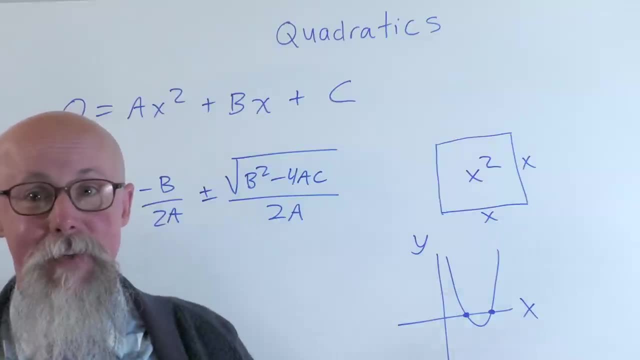 through this. once for plus, get that answer. once for minus, get that answer. there we go. but also, since i'm square rooting something, uh, we're just, we're going to stick with the real numbers here, and if i have a negative value under this radical, then there's no real solution. so you know. um. 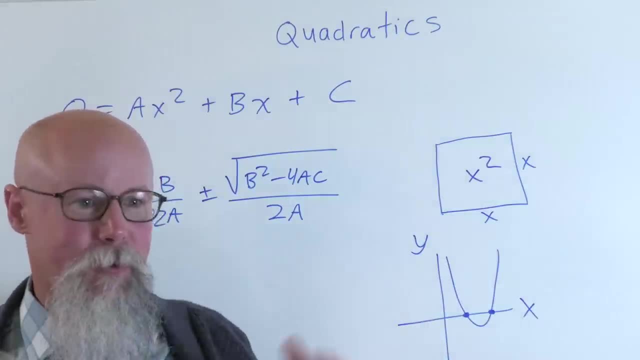 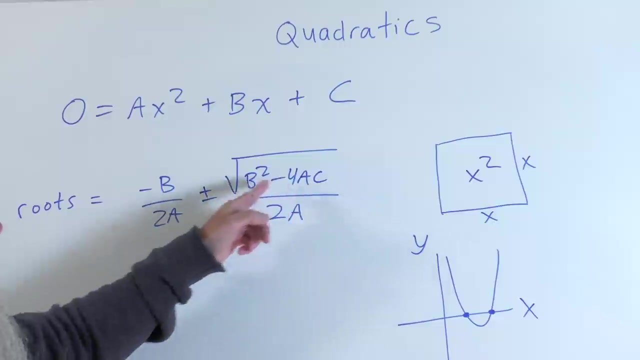 we could get into a imaginary numbers and you know it's not real solution. but why should we let that stop us? but for our purposes we're not going to worry about that. we're going to say that if it's negative, then there's no real solution and we're going to just stop there. so in doing this, i would often test. 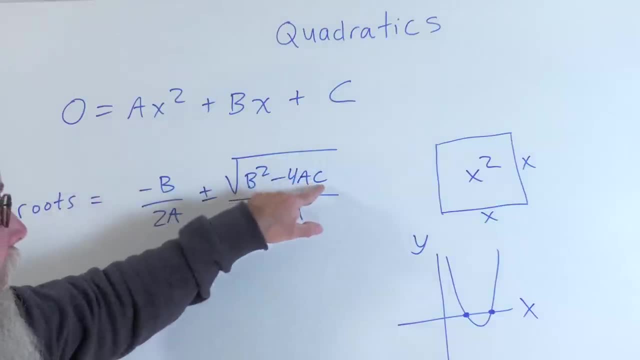 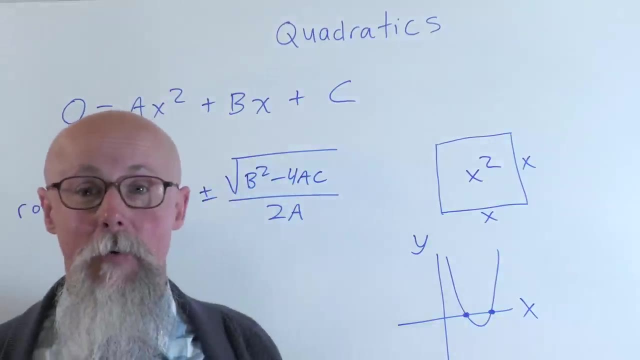 this. we call this part under here the discriminant, and i would often test this. you know, b squared minus four, a c does that? is that zero? actually that can be zero, which is fine, but if it's negative, then that would be plus or minus zero. you know, that means it would have one. 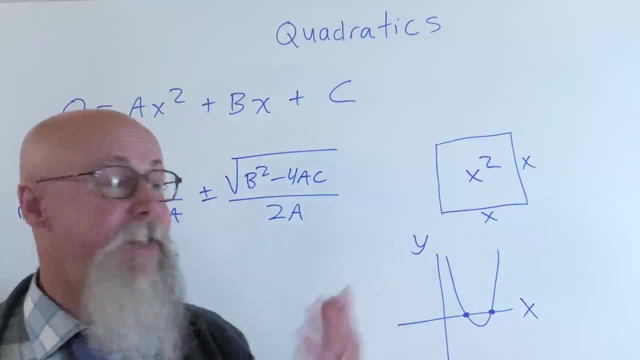 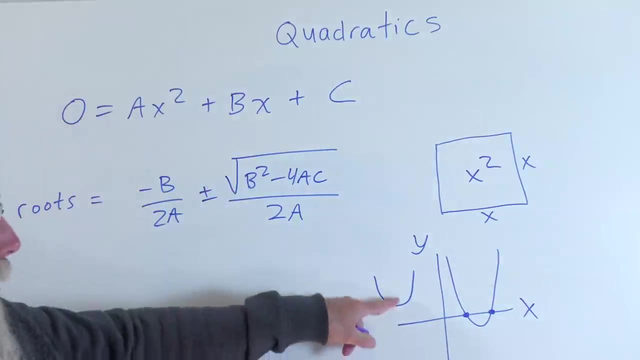 root, it would just touch the x-axis. that's fine. but if it's negative, then that means i have no roots and i would have a parabola that just never touched the x-axis. so that's. that's perfectly fine. it's possible, and in that case i would test that first, and if i knew that, then that would save me. 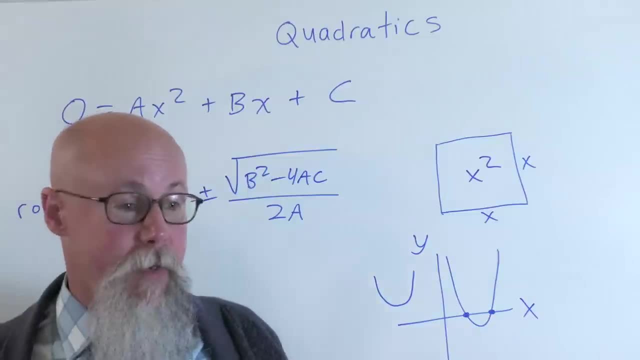 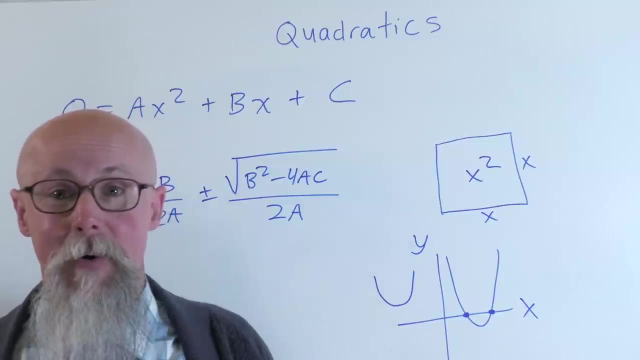 some time. you know not having to do all this because you know if we did this old school and just doctored it all out, you know right writing in the notebook. you know sometimes it takes a while. we're going to look at how to make this a lot easier. you know writing the code we're going to put. 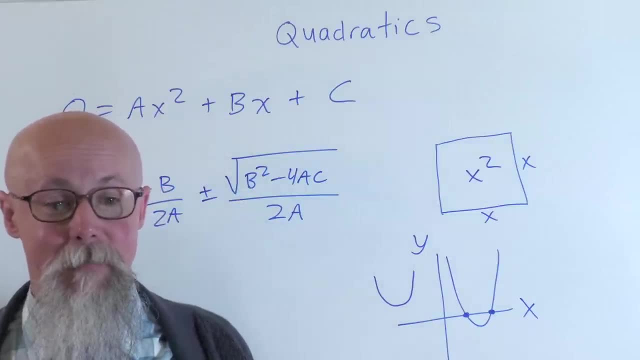 these formulas in, and then we're going to find the roots in the vertex. you know, maybe we'll even graph them too. so this is the formula. and notice: in math they're both have the same denominator, so i could- i could- make this all over one denominator. like that works out. 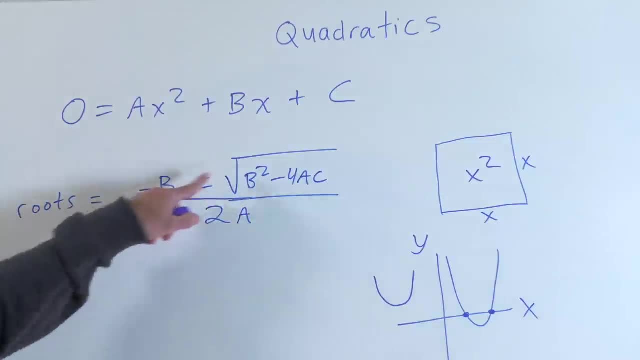 you know, do the adding or subtracting in the numerator all over one denominator and mathematically that works out. you know it's another way to write it, so this is very often. this is the quadratic formula as we would often see it just like this: all that all over 2a. 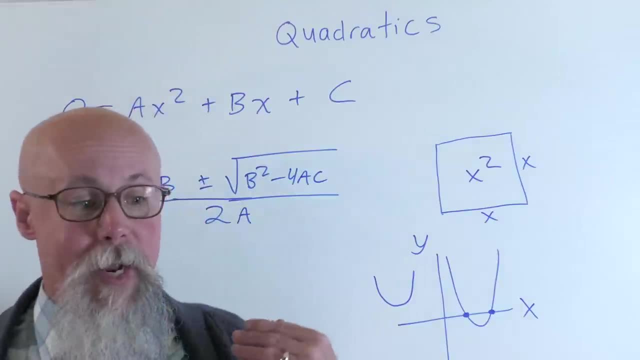 and so for. as complex as this could be, there's only a few formulas. all right, i see this: i get a b and c formula for the vertex, and then i get a b and c formula for the vertex, and then i get a b and c formula for the vertex, formula for the roots. we look at graphing it and then you know, then we can. 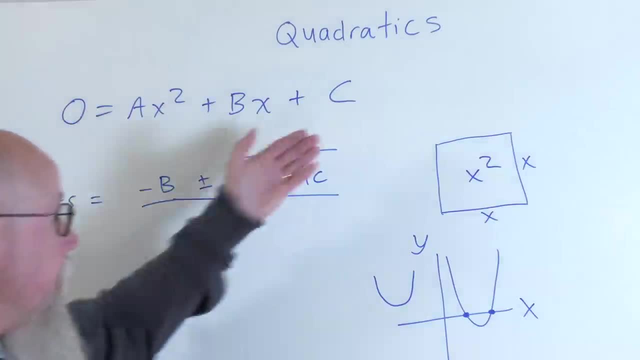 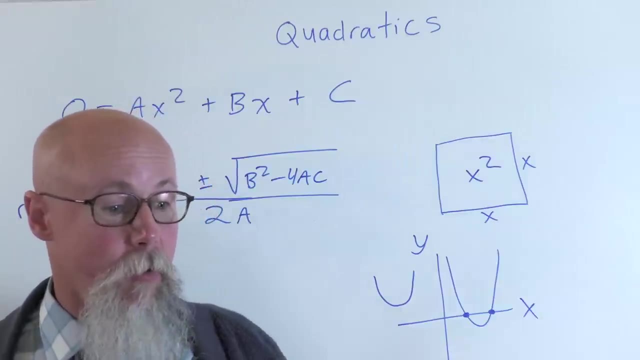 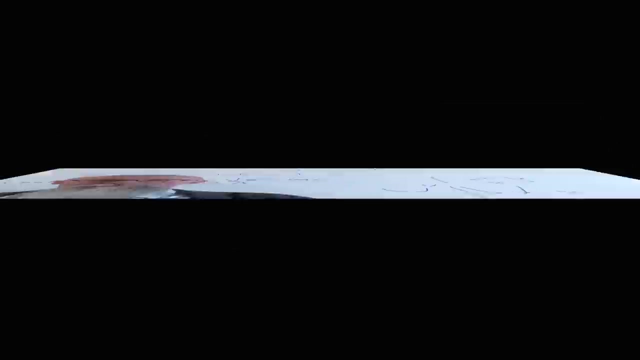 look at some of the applications, but this is where this is kind of the essence of looking at quadratics here and so now let's take a look and we'll go into some other. um, well, you know how to solve these formulas and everything, so let's take a look at the code. so, solving a quadratic equation. 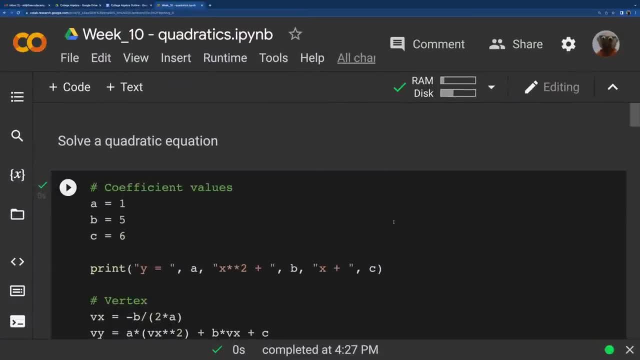 is much easier with code, because all the formulas that we were talking about are that we would work out by hand. we're just going to put them all into the code so you can just define a, b and c once and then run those values through all the formulas you need and output your answer. 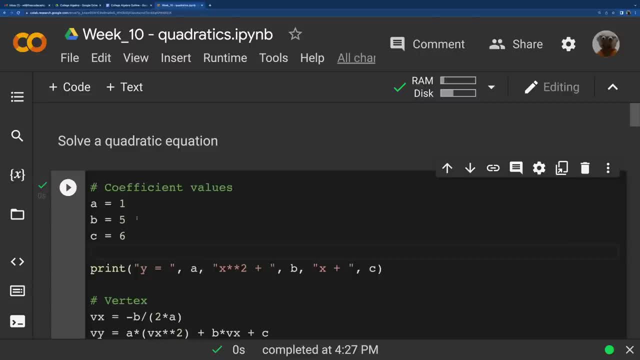 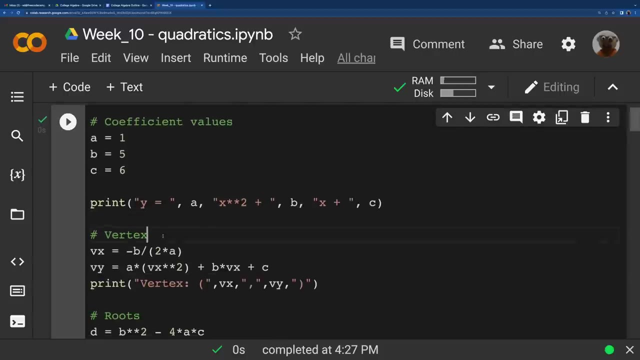 roots, vertex and whatever else you need. so i just picked some values here that work out uh nicely: a, b and c. and what do we want to do? let's first of all just print it. so we'll print out what our function is. then we'll calculate the vertex. so notice vx. i call the variable and that's the. 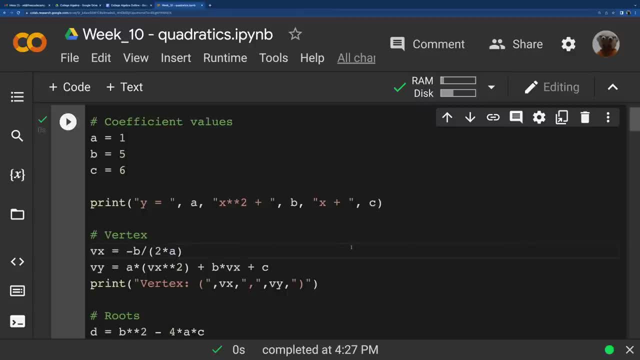 negative b over 2a. that's going to calculate the x value and python does no order of operations. but this 2a does need to be in parentheses because it is the whole denominator. so we get that x value and then we're going to take that x value and plug that in for the y value a times. 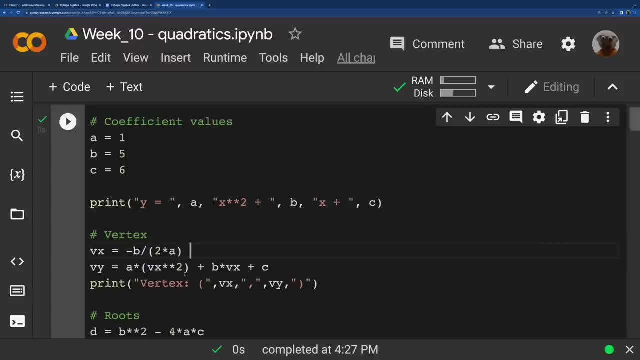 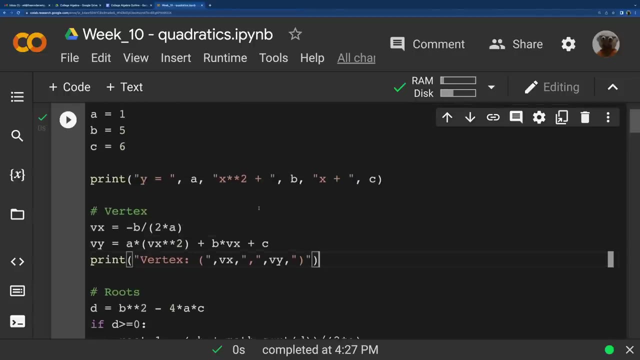 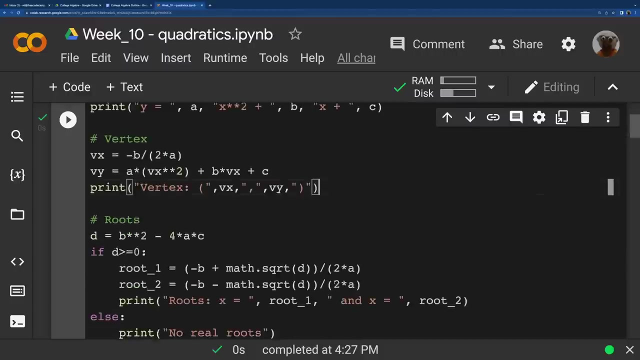 and my x value, vx, and then square it plus b times vx plus c. so i get, i plug all that in, get the y value and, just like before, i'll print it now. um, there we go. we just print the equation. now we have the vertex as a point and we'll go on to. 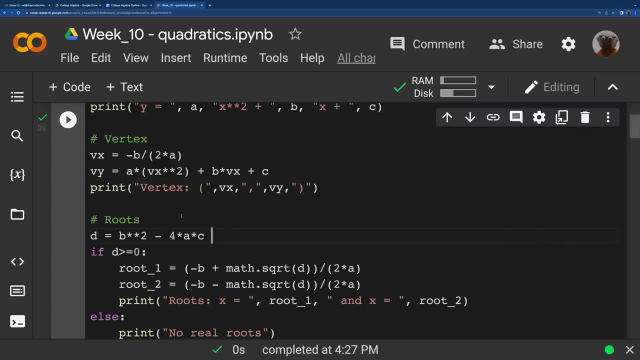 the roots and the roots. remember the quadratic formula d. it works out a, b, c, d, but it's actually d is for determinant here, that's the part that's underneath the square root, because if that's negative, then i won't have any real roots, and so i'll just define d as that part under the square root, b squared minus 4ac. 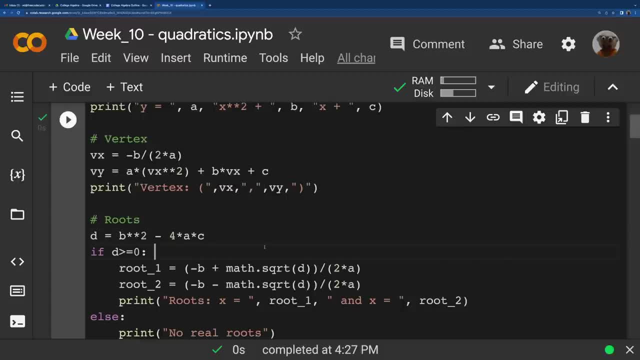 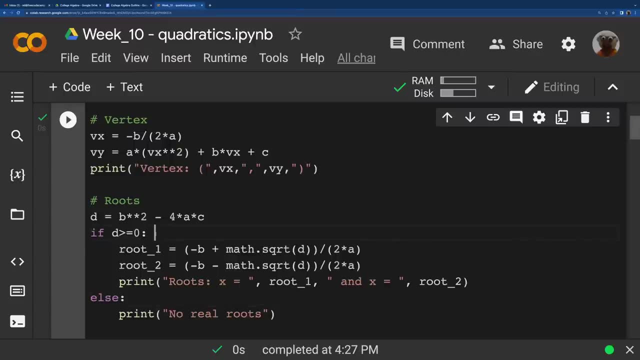 and then i'll test it here- if d is greater than or equal to zero, because if it's not, then i'm going to print out no real roots. so if, as long as it's greater than or equal to, then we're going to calculate the roots and remember the. 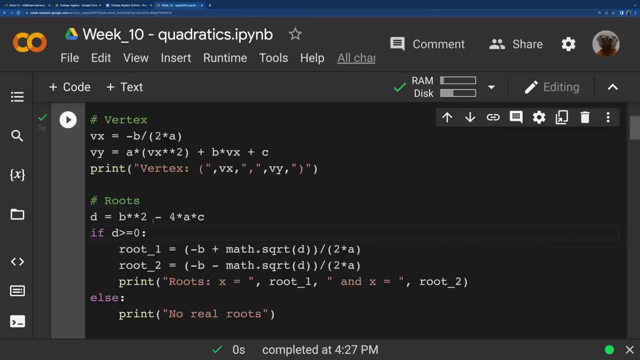 the roots and then we're going to print out no real roots. so we're going to print out no real roots and then we're going to do the quadratic formula. so since i already figured out d, i'll make use of that. so negative b plus or minus. so we're going to run through this twice. for the first root, negative. 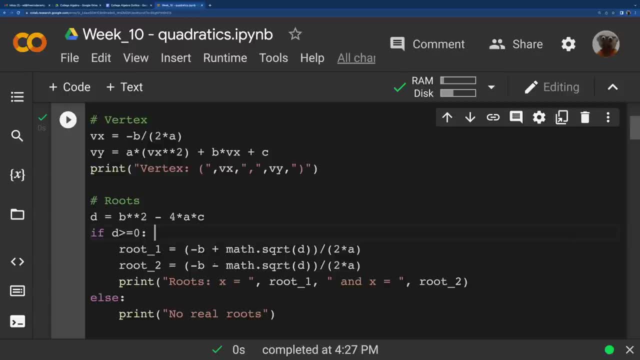 b plus the square root of d and then all that's over 2a and notice parentheses for the numerator, parentheses for the denominator and then the second root, negative b minus the square root of d. calculate the roots, print it out, or you know no real roots, if that's the case, 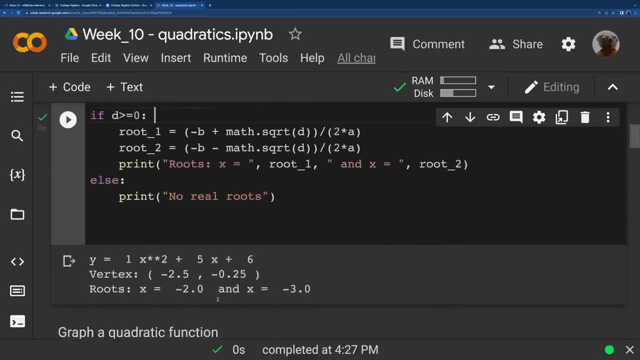 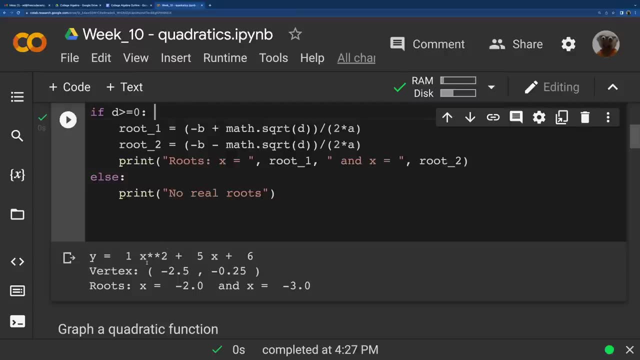 and there we go. So I actually already ran this. and what do we have? y equals so 1x squared plus 5x plus 6, and then we have the vertex: is this negative 2.5,? 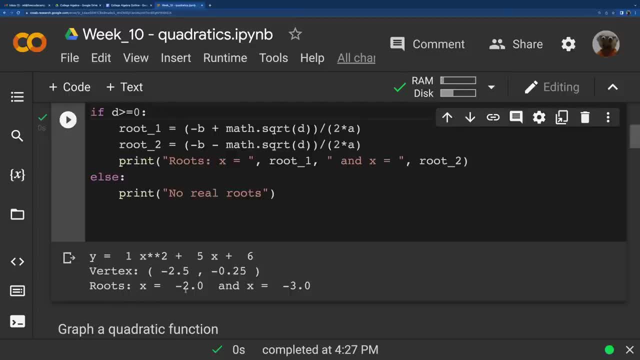 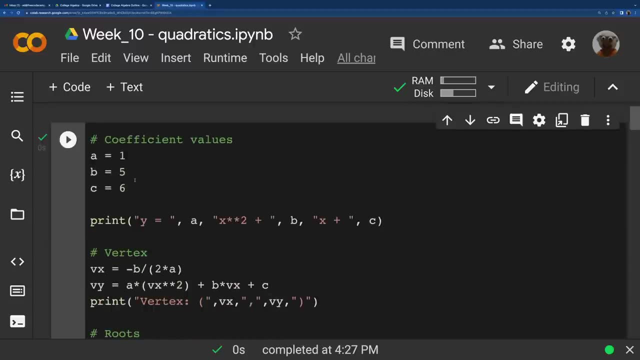 negative 0.25, and then the roots: x equals 2, negative 2, and x equals negative 3.. So there we go, If all you need to do is solve it. it's nice to have all these formulas at the. 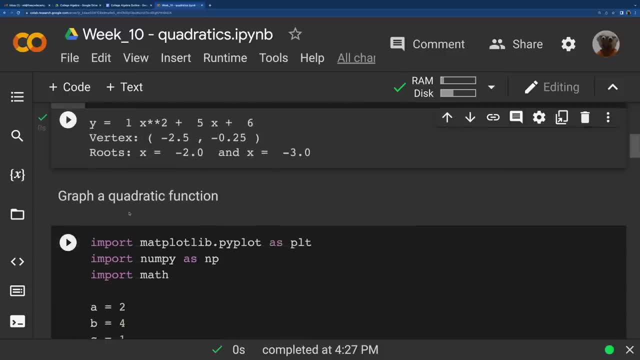 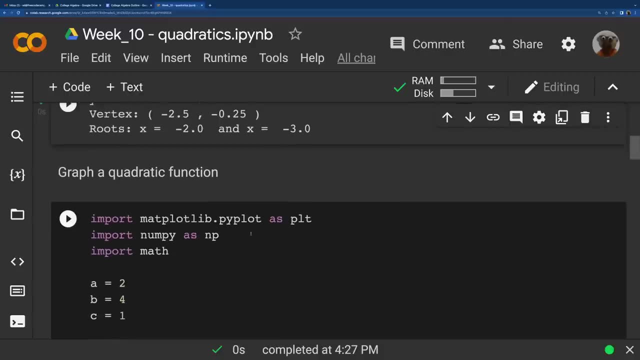 ready, just change a, b and c and run it again. So if we want to graph it also, we can do everything we were doing plus the graphing part. Remember our imports for graphing that plot library numpy. I'm also going to import math for some things that we'll do. I'm going to define a. 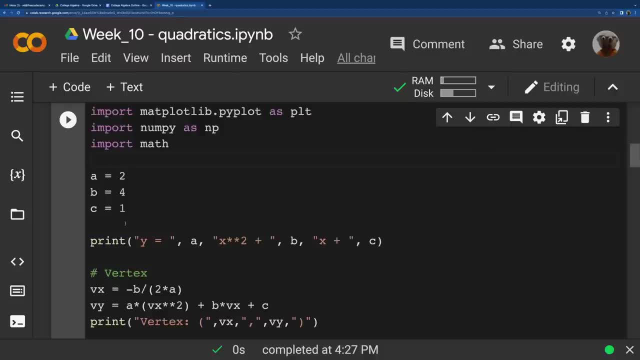 b and c. So I'm going to do a, b and c. I just pick different numbers here and I'm going to print out a, b and c. So this part is very similar. I'm going to print this out, calculate the vertex, print that out and now we get into. 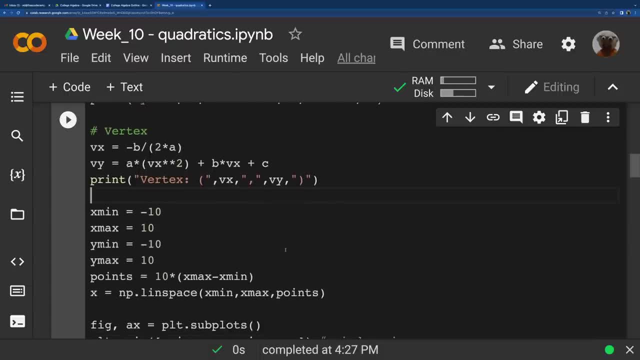 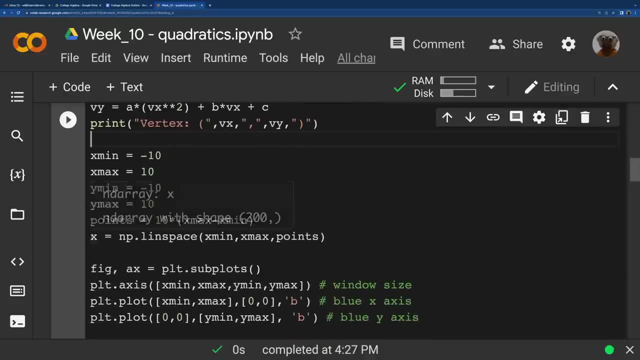 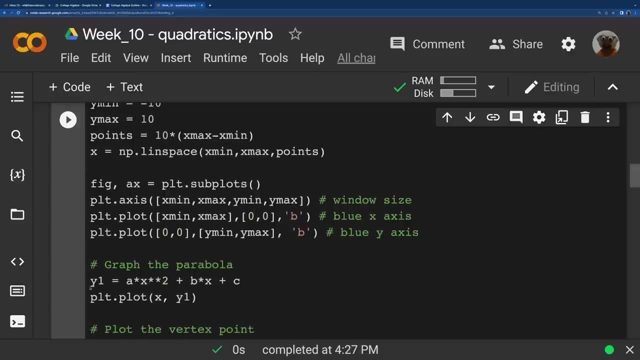 the graphing. So notice, I didn't do the roots yet and we just have x min, x max. you know everything else we were doing for graphing: define the x values, set up the plot and now I can graph the parabola. I just called it y1, even though I probably won't have a second y value. 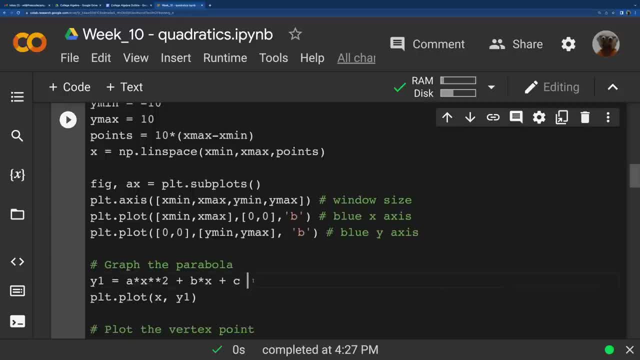 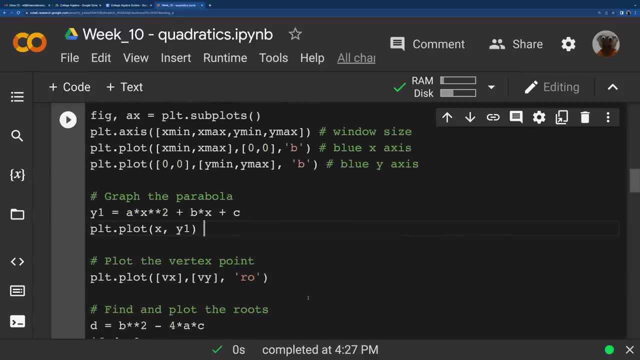 here ax squared plus bx plus c. There we go. I'm going to graph that whole parabola and then that's y1.. So I'm going to plot x and y1. Then I'm going to plot the vertex as a point. 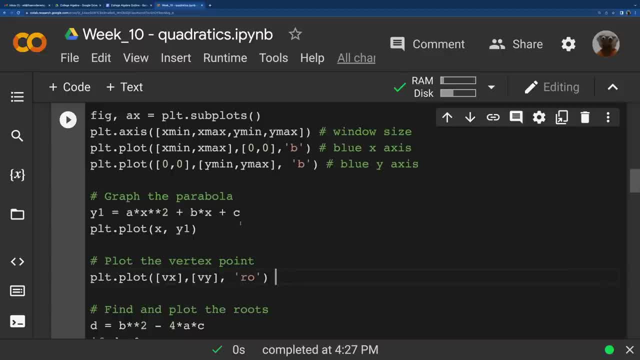 So I put this all down here for the plotting Parabola, the vertex point, and then notice this one up here: by default it's going to be a line, And here I'm defining two arrays, each of them with one item, and then that's going to be a red. 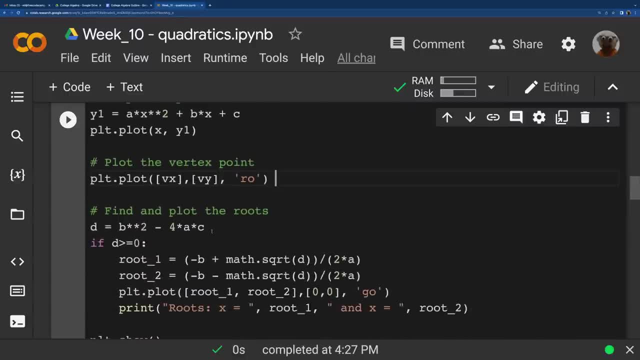 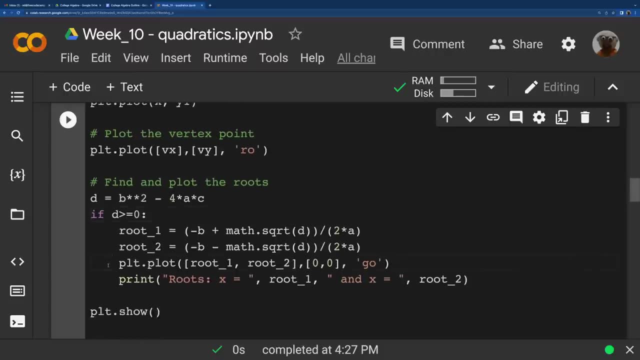 dot. So then we're going to find and plot the roots. Everything we were doing with calculating the roots from before. but I'm going to add this one line here: pi dot, plot, And once I get the plot, I'm going to plot root 1, root 1, 0, and root 2, 0.. And remember, you know the array of. 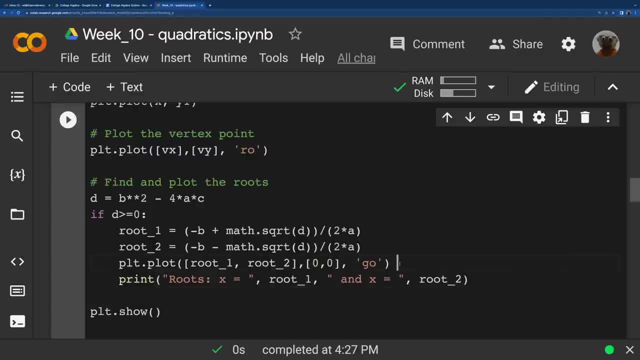 x values and then the y values, And this one is going to be a green dot, So that's why it's going to be a green circle. So I'm going to plot that and then I'm also going to print out the 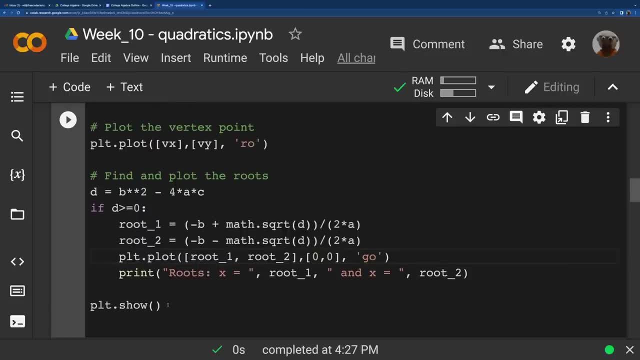 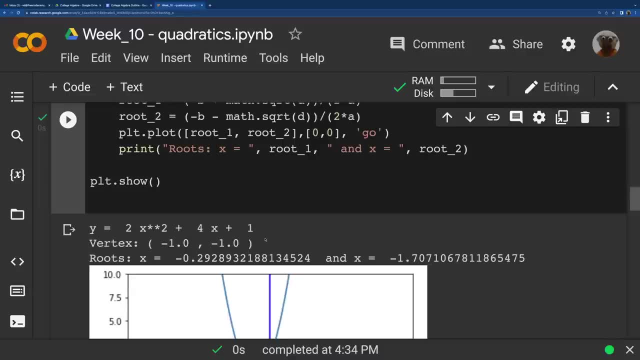 roots, because I want to see that too. So when we have all this and then we run it, it'll have your equation here. There we go: x squared plus 4x plus 1, give you the vertex. 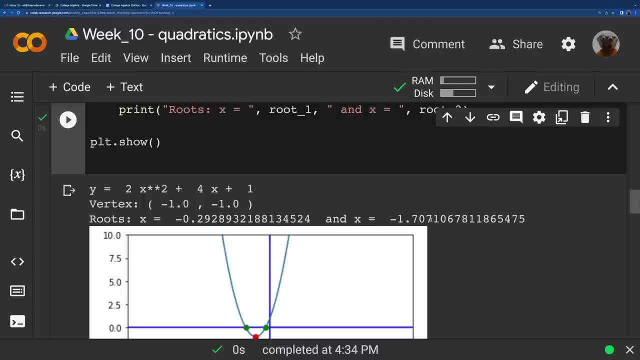 and give you the roots. Now, these roots are irrational, You know. that's why it gets this wacky decimal. We could, you know, do quite a few more lines of code to get to the wacky radical answer, but we're not going to worry about that now. That's. 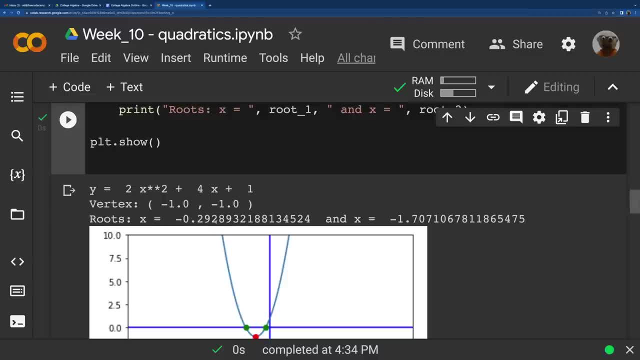 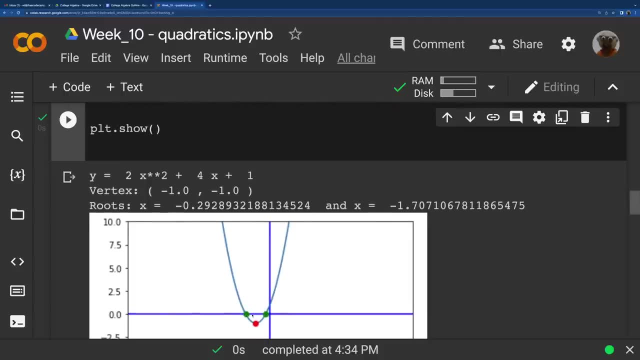 perfectly fine. If you're writing this down somewhere, you might round it to a couple decimal places. But here we go. We plot the vertex as a red dot, the roots as green dots. you know, see where it crosses the x-axis, and then we graph the parabola. 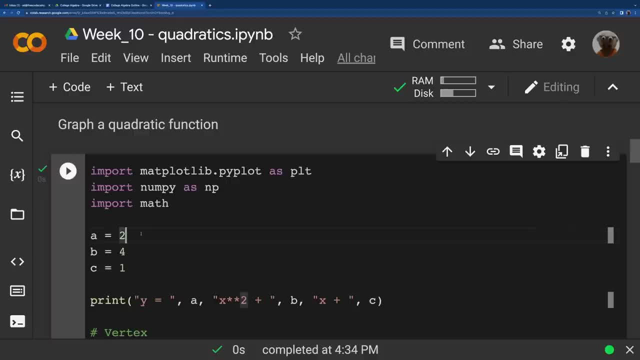 And so I can redo this. Then let's just try these numbers that we were doing before: 1,, 5,. there we go, 6, and that's all we need to do. Change a, b and c. 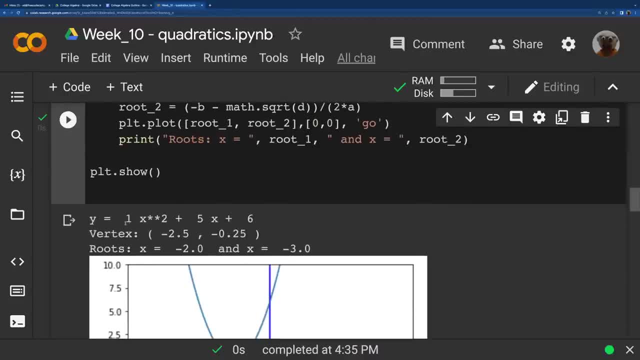 and it'll run through and calculate all this. There we go: x squared plus 5x plus 6, and here's the vertex: negative 2,5,. negative point: 0.25.. negative 0.25, and then the roots. 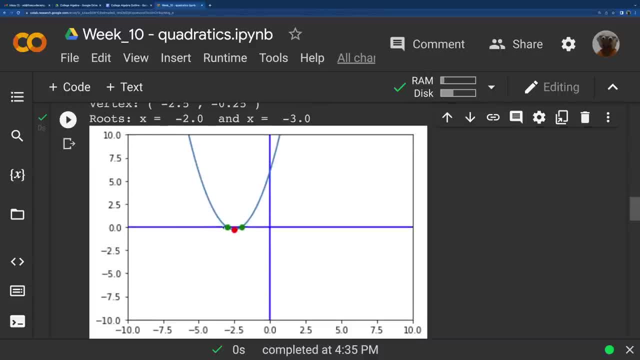 negative 2 and negative 3.. There we go. Now, there we go. Negative 2 and negative 3 are where it crosses the x-axis and see, the y-value of that vertex is negative 0.25.. So it's just below it, but just. 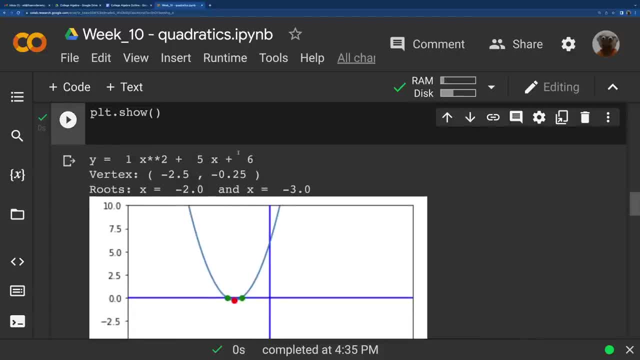 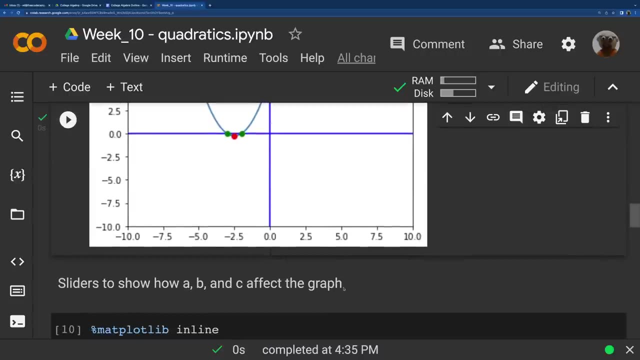 barely. And there we go. So we can plot our quadratic formula, we can graph it, we can get our roots and our vertex and for most things, when you're solving quadratics, that's what you want to do. So let's take a look at. 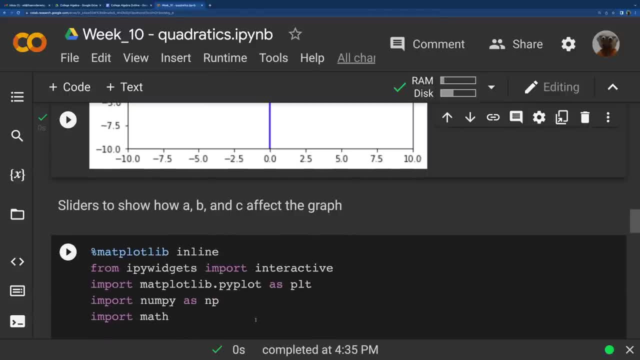 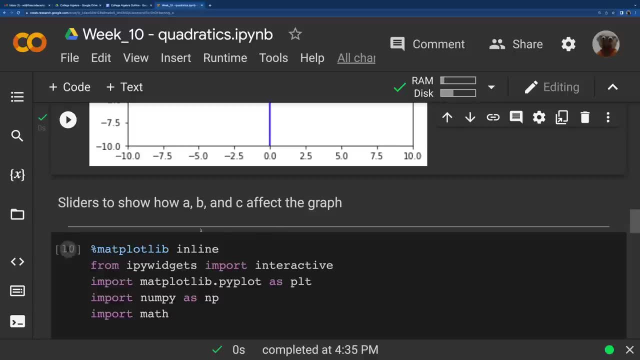 how a, b and c actually affect the graph. So I'm going to show you some sliders here and that's going to come up again in one of the other notebooks. So how a, b and c? So the first thing is we're going to import this and 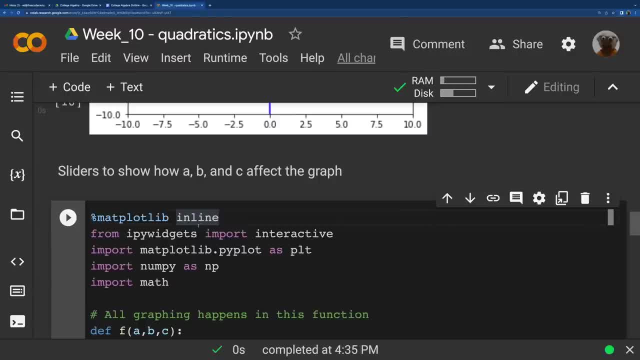 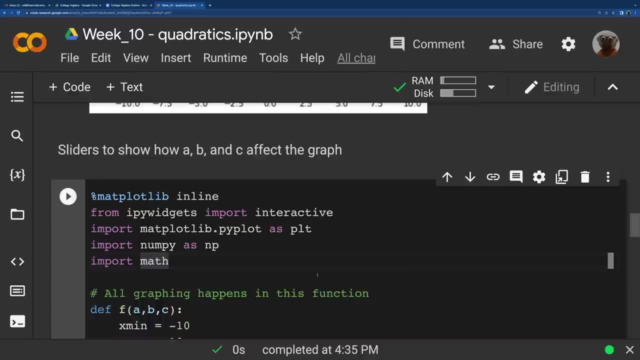 just that way, matplot inline and we're going to write that first and then we're going to import these widgets and interactive and then the same other things we're going to do with the plot. So the way that these widgets work is we're going to 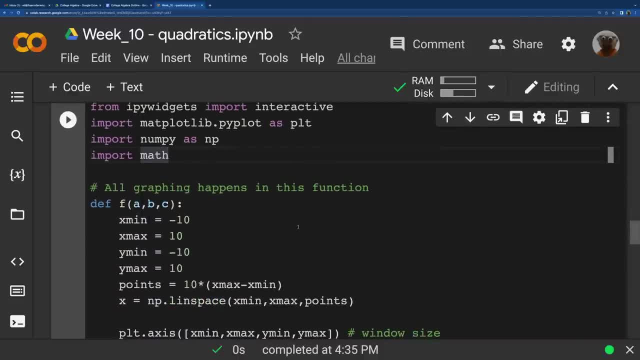 put all the graphing in this function. So now we're going to connect again with functions here. I still defined it just as f and that's because later on I wanted it to be a short name for that line. but we'll see. 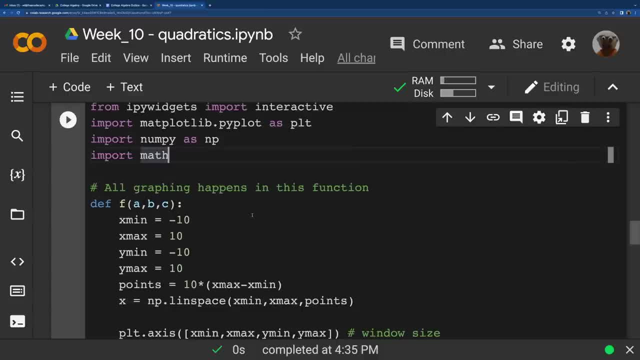 So I'm going to define this as f, but it's the function of a, b and c. I'm going to take those three things- a, b and c- as inputs. Now you could always make this, say quadratic and do everything. 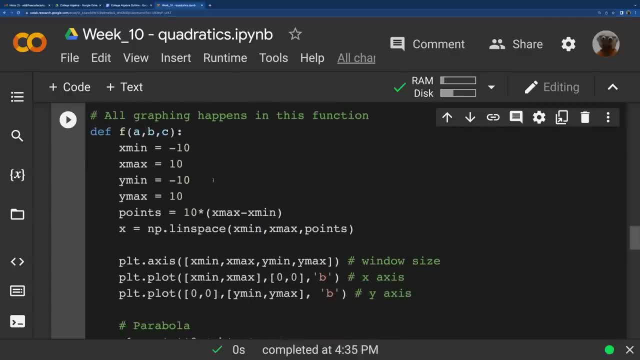 that you want to do with the quadratic Roots vertex. we could actually take everything that we were doing before with the plotting and with the solving and put all that in this function. At that point I would call it more than just f. I might say quadratic and take the argument. 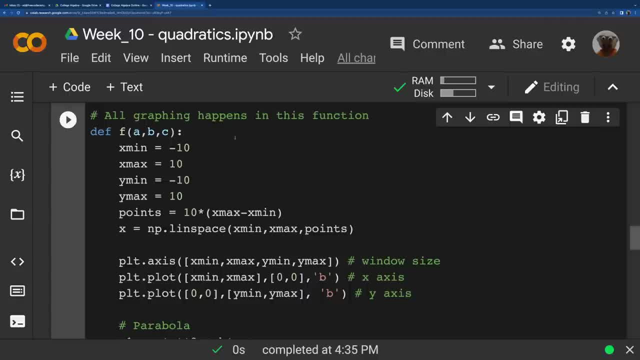 a, b and c and do everything you need. So kind of cool that you can do that. but here we're just going to focus on the graphing. So my function there we go: x min, x max, all those I'm going to. 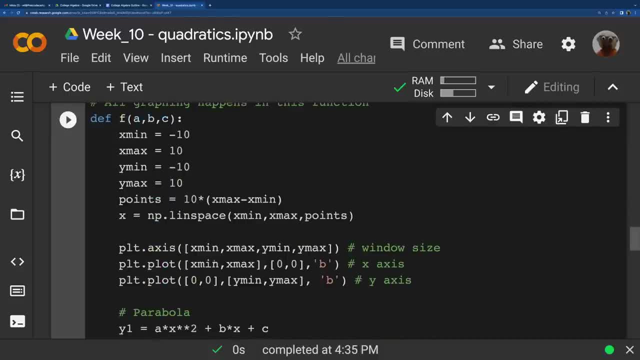 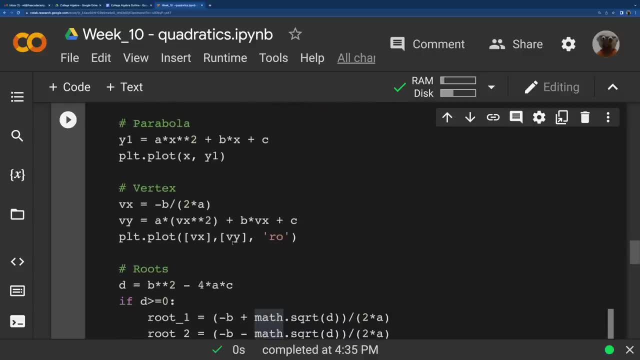 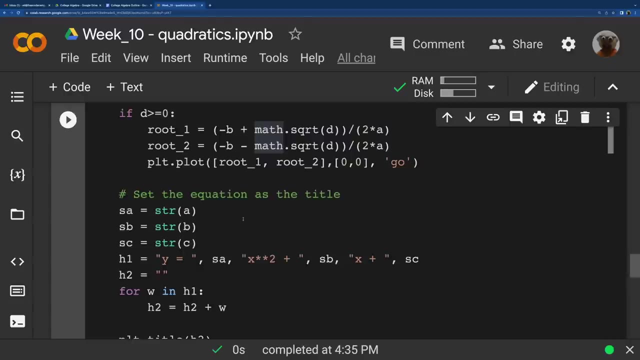 define all these things for graphing. Remember a, b and c would be the inputs, so we would have those, And then plot the parabola, plot the vertex as a point, plot the roots as points, And there we go. 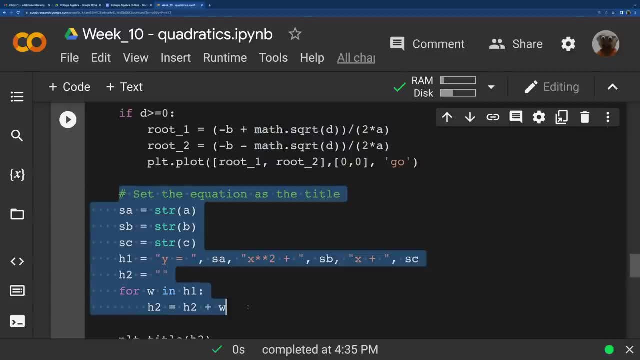 This, all of this here is really just extra for the sake of setting the equation as the title of the graph. I did that instead of printing it out, which I guess we could have done, but I wanted to show you we could set it as the title of the graph and the title needs to be a string. 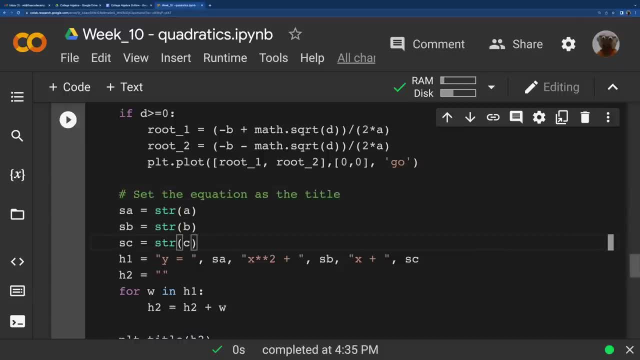 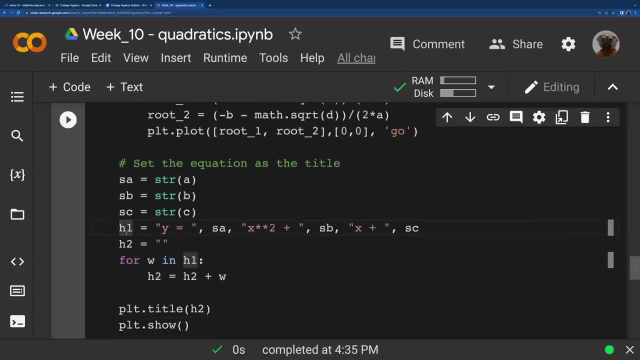 So here I'm going to take a, b and c, convert them all to strings. Then I'm going to take all of this, and I was. you know this doesn't necessarily connect with HTML, but I was thinking of that. 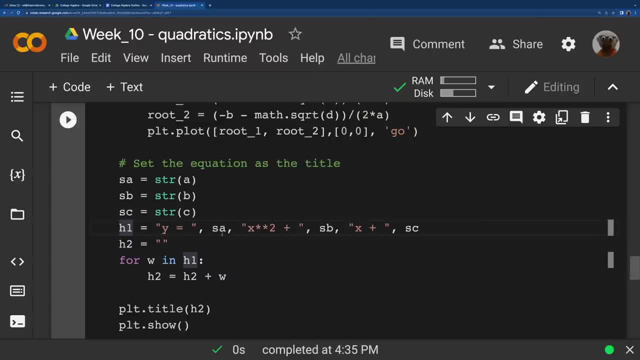 h1 for the heading. so I'm just going to combine all these or concatenate all these, that exact y equals combined with sa, that string, and I'm going to combine all these as h1.. But if I just leave it at that, 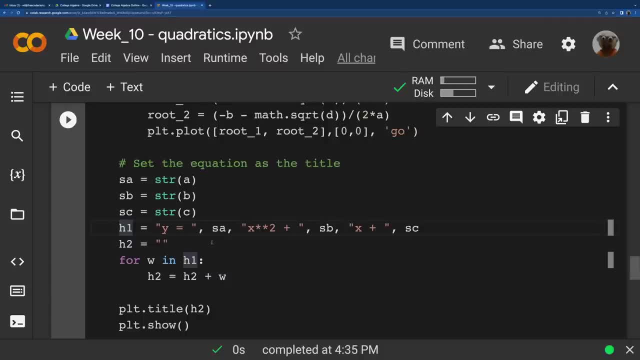 it'll still display in a weird way as the title. They'll be like extra quotes and I don't like that. So I'm going to just find this other one, h2, with just blank with quotes, and that's going to be a string And I'm going to loop through this. 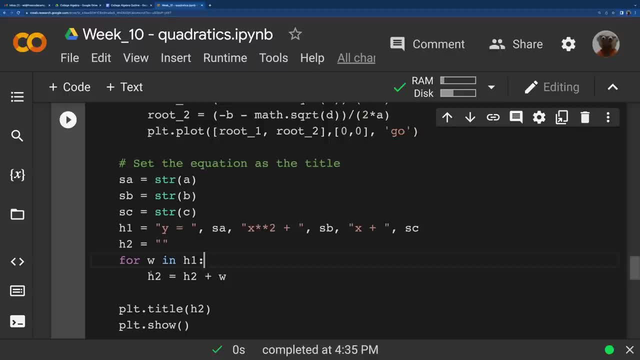 for w in h1,. you know w like for word in h1, and then h2 equals h2 plus w. So I still had to convert these to strings, put it all together as h1, but then I still needed to put it in h2. 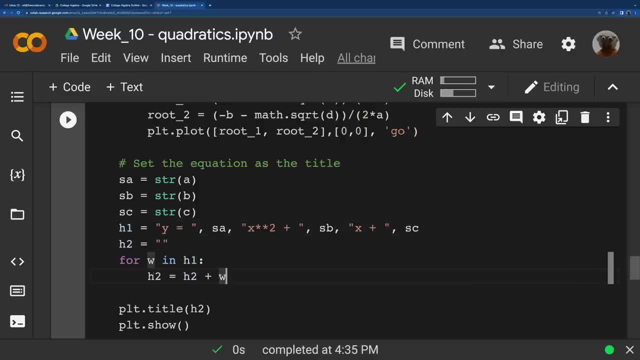 if I do it this way, combining these now, h2 is a nice unified string without a lot of extra quotes, And so that's you know. again, it's a lot to just. it all leads up to the sake of. for the sake of. 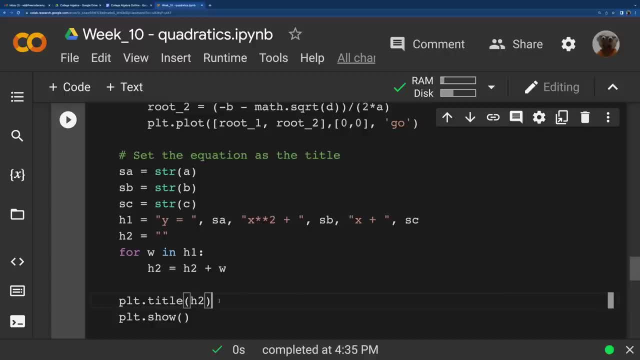 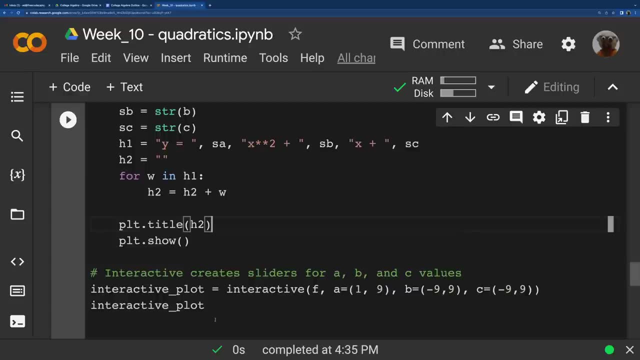 putting this as the title. Okay, And you know, we'll see. Hopefully, you know it looks nice and you know you see how that was. you say, oh, that was worth it, All right. So here's where the interactive comes in. So 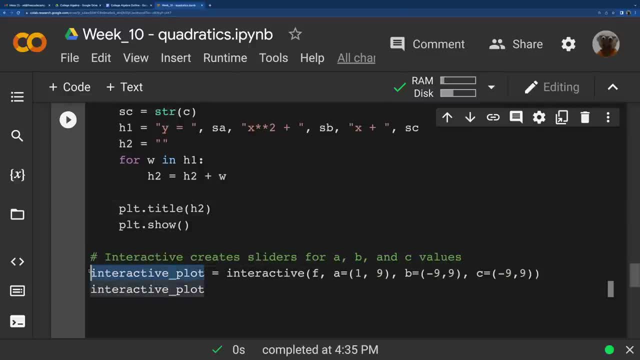 we have this interactive plot. Now, that's just the variable that I chose, interactive plot. But here's what's really happening, this interactive function. So if we take a look at this, so it runs this function f. 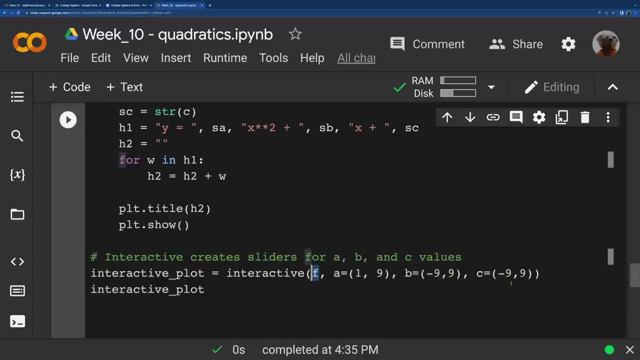 So that's where the name of your function goes And that's where you see how long this line got. I wanted this to be short, So I just that's why I called it f, So it runs this function. 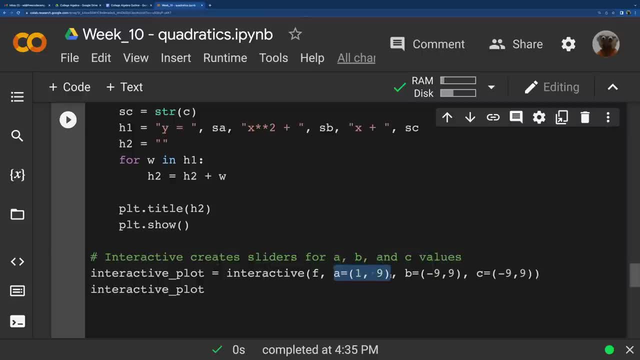 And that function. and then it defines: a with a range from 1 to 9. b with a range from negative 9 to 9. And c, also with a range from negative 9 to 9. a: I started at 1 because 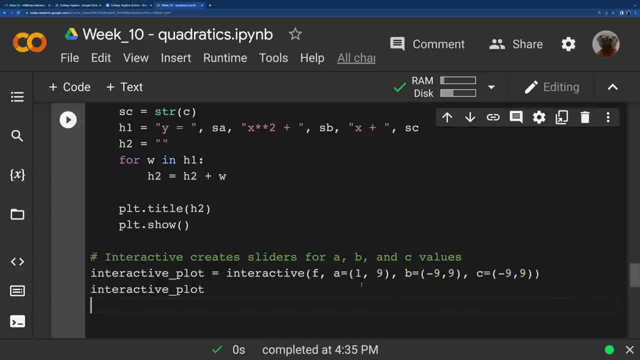 if it was 0, that's actually not a quadratic, and I want to illustrate quadratics, And so I'll start at 1.. So we just define this interactive plot And then notice this as the last line of code. 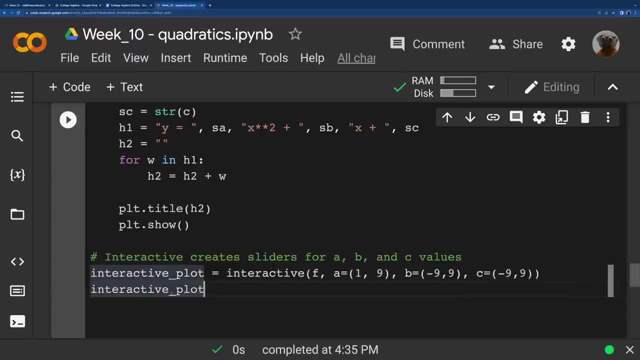 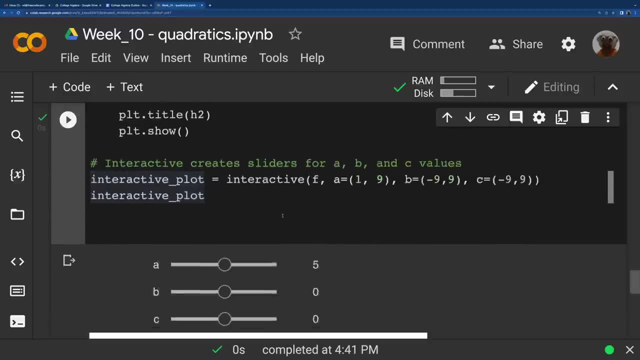 Then if I just say interactive plot, it's going to print, it's going to run that. So we'll see this interactive, how that makes the sliders here. There we go And it default shows them in the middle And see this is. 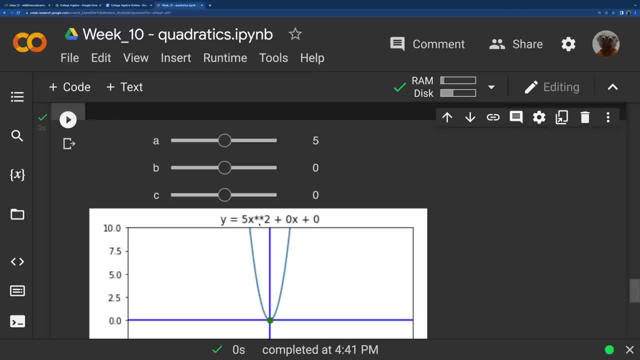 what I wanted it to be, That when it starts out, you see the title of the graph: y equals 5x squared plus 0x plus 0.. See, that's it Just. and if I go, if I make that, 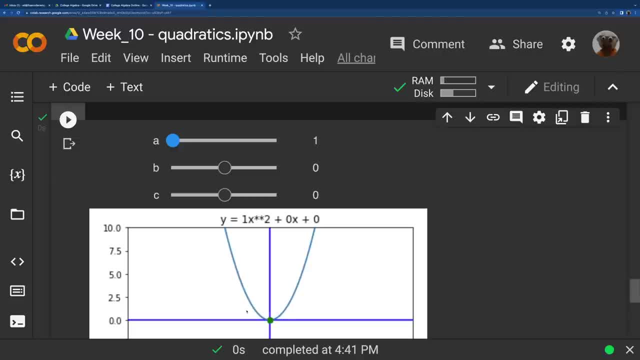 down to 1,. this is the parent graph, the most basic parabola. You know x squared and I don't have to put the plus 0, but in this case it's going to write that every time, And then we can see what happens if I move. 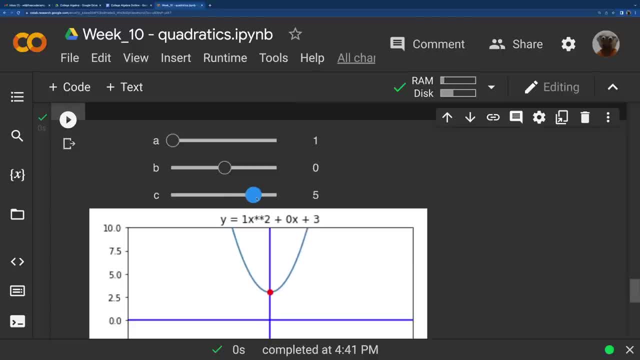 c. You see I can move c and it'll adjust the graph. it'll adjust the title Of the graph. there we go, And then we can see what happens. if I move b, You see It moves it along here. 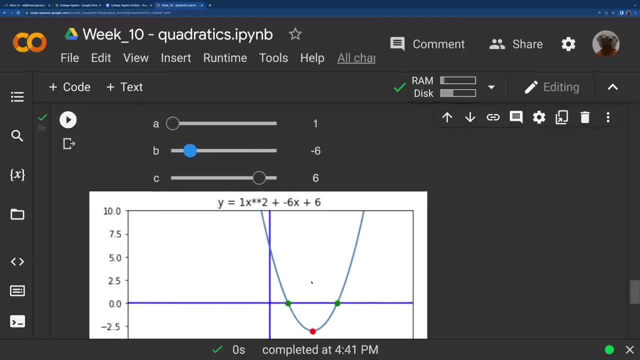 And now it got to this point that now where it is, I do have roots in the vertex that I can display, And then, if I have, I can see where b move that around affects this whole graph, and I can see then how a affects. 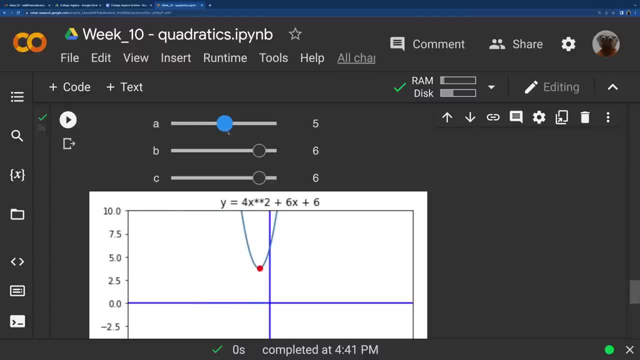 the whole graph. so we see some different things that we can do, and all these are going to be accessible to you. you can tinker with these, but this is all you know. it was just I wanted to show you this interactive. you can set up sliders and, in this case, to display the display, the graph. see the roots in the vertex. 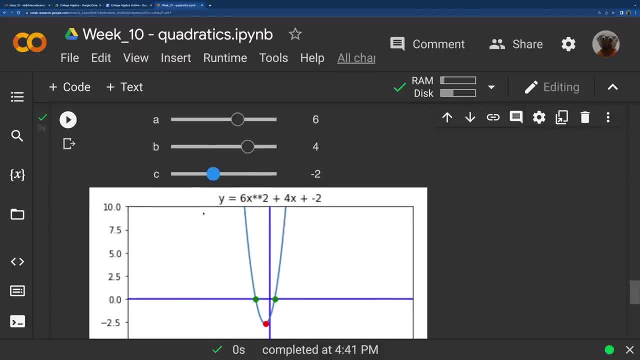 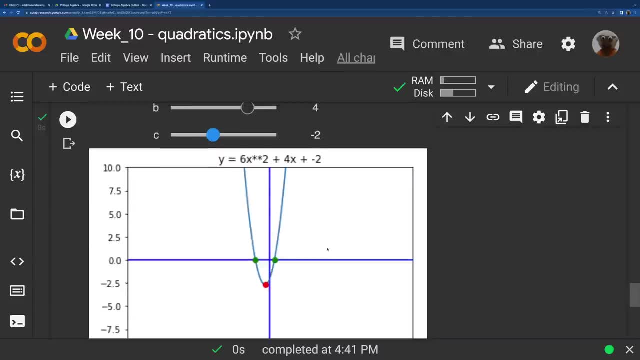 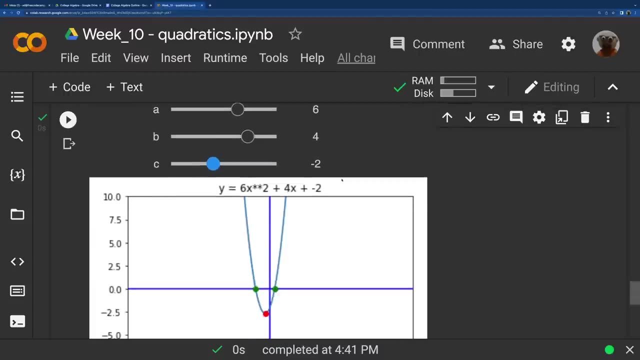 you see, and I move that down so we display the graph, see the roots in the vertex and adjust it with sliders. you can see how a, B and C affect the graph. so knowing this and being able to have all this code at your disposal, you can really see you. 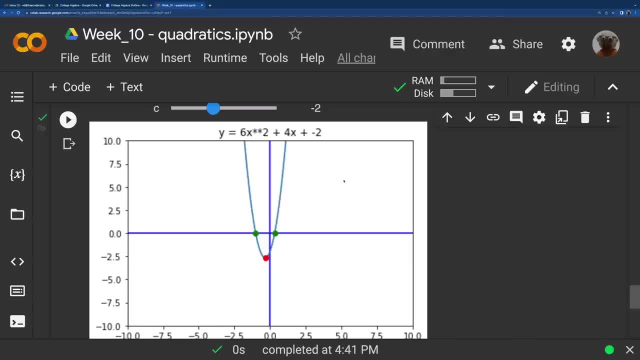 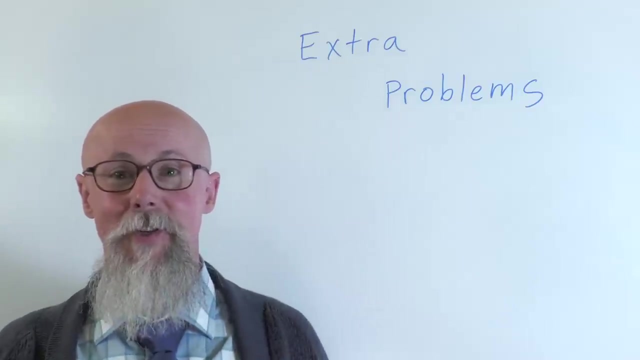 know most everything that you're gonna need to do with quadratics. you know find the roots in the vertex, see the graph, and you know adjust it and you know do some other things. so there we go: this and some practice, you'll. you'll know quadratics inside and out now that we've worked through the core skills in this. 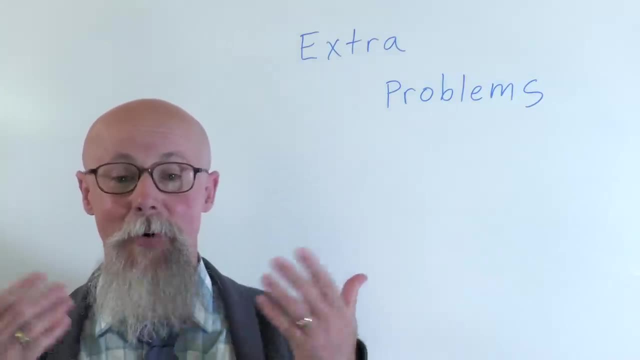 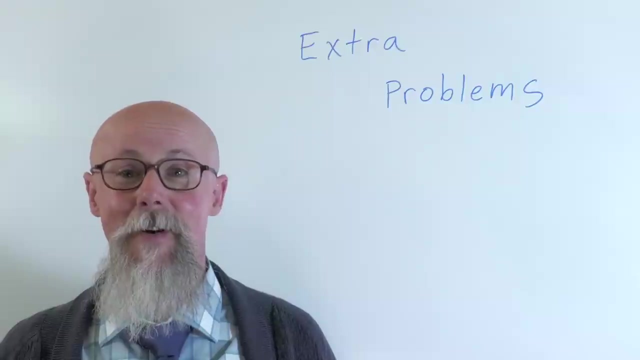 unit. let's look through some extra problems, and I'm going to work through extra problems using the Colab notebook so you can see how you can apply these resources that you're building and use the use these to solve problems that might come up in a textbook or in day-to-day life. so we're going to go. 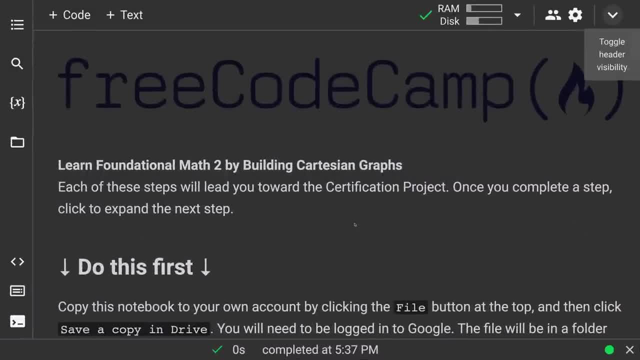 through some more extra problems here. so here we're gonna walk through the foundational math certification 2, and if you have not already done it, please, Please, give this a try on your own. This is for if you've already done that and you're stuck. 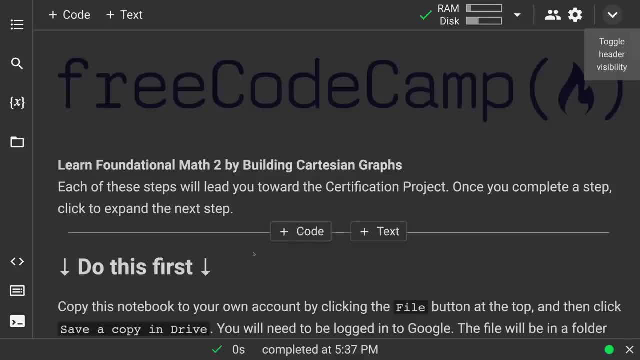 or if you just had a question about one of the parts. we'll hopefully answer all those And, just like the other certifications, this one, you're going to make a copy and put this in your Google Drive. So file, save a copy in your drive. 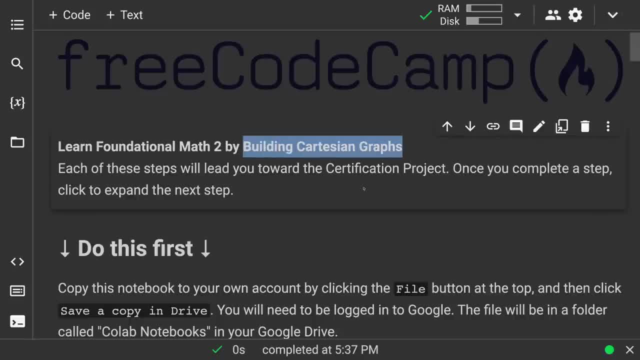 And this one we're going to focus on building Cartesian graphs. So most of this is going to deal with graphing. We're going to look at some different functions and what you can do with that. So make a copy in your Google Drive. 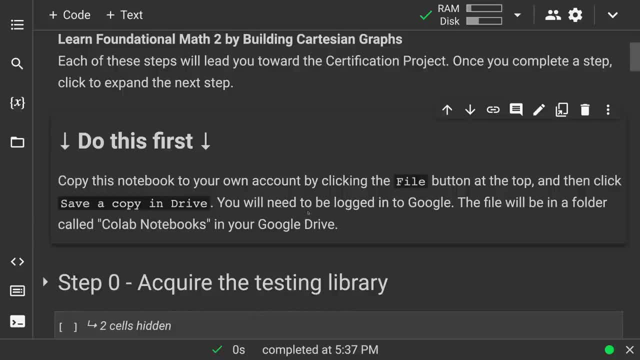 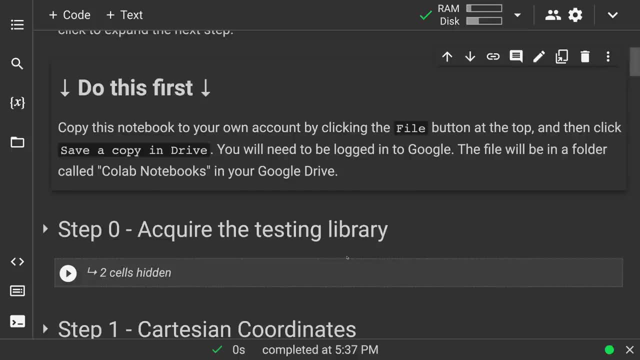 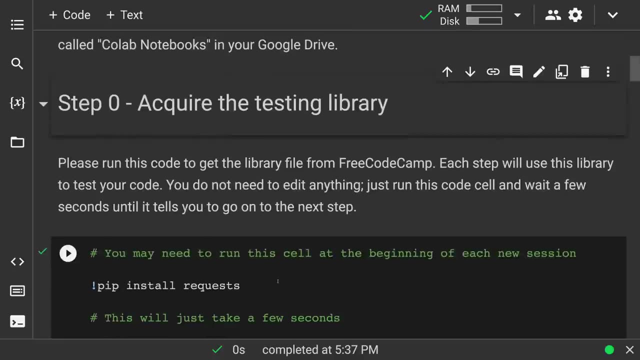 It might be in your Google Colab notebooks folder where you can put it wherever you want. And now hopefully you know I already did that, So hopefully you're now working from your copy and we need to acquire the testing library, So the code that you write, just like the certification one. 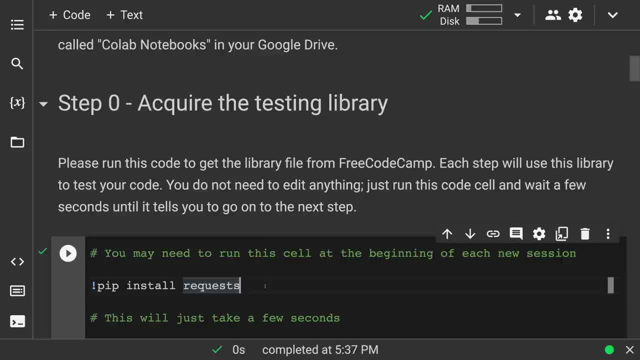 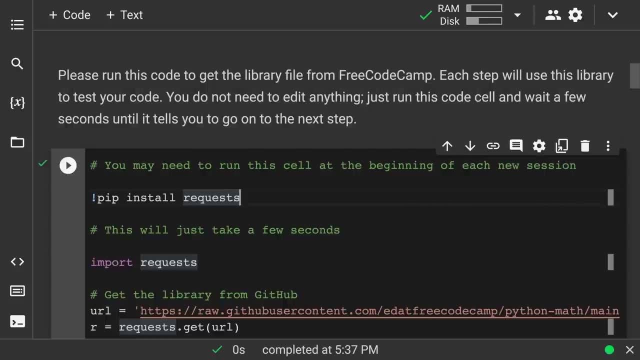 the code that you write when you run it. it'll run through these tests to see if the code is what it's supposed to be and then give you some feedback. So this first cell: you don't need to do anything, And you might just take note of what you need to do here for future reference. 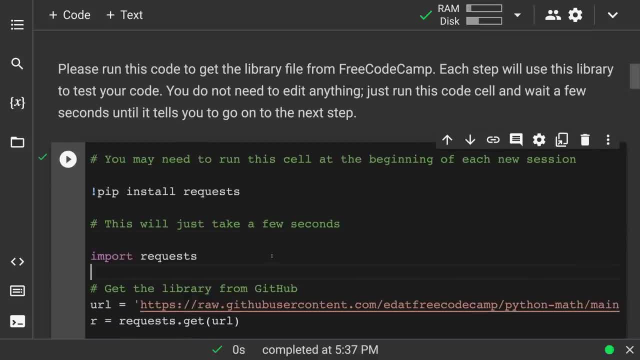 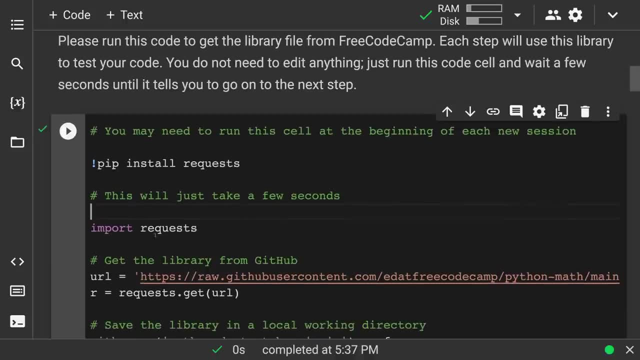 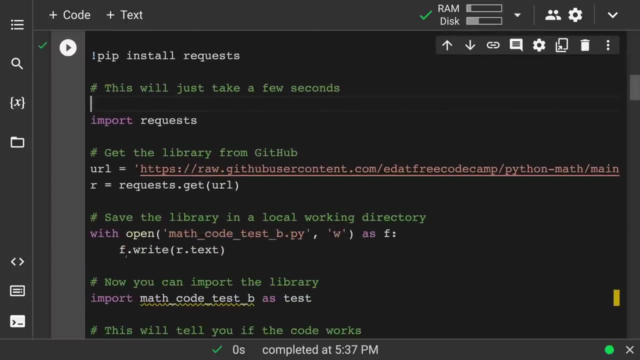 in case you want to have your own custom library that you include in your Colab notebook. So this custom library it's on GitHub and this code is going to get that and save it here in a local working directory. So you will need to run this for each new session. 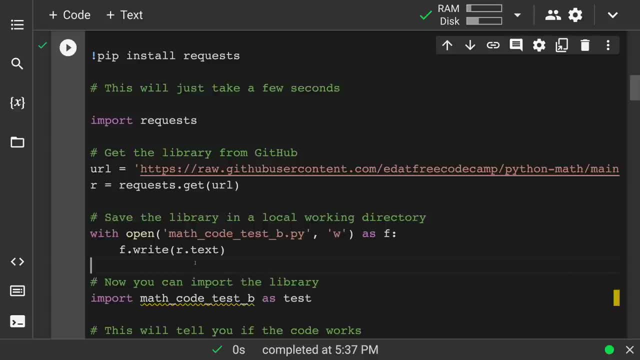 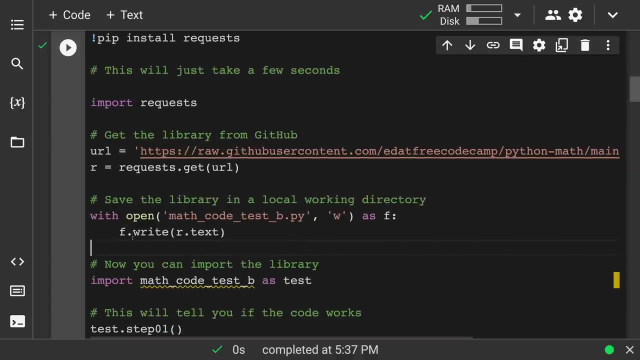 As I mentioned before, the session will time out because of inactivity after 30 minutes at the most, Or even, if you're busy, 12 hours. it'll time out Each new session. run this and it'll go through and then import the library. 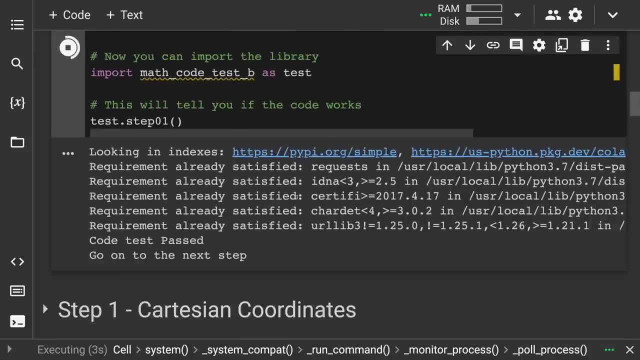 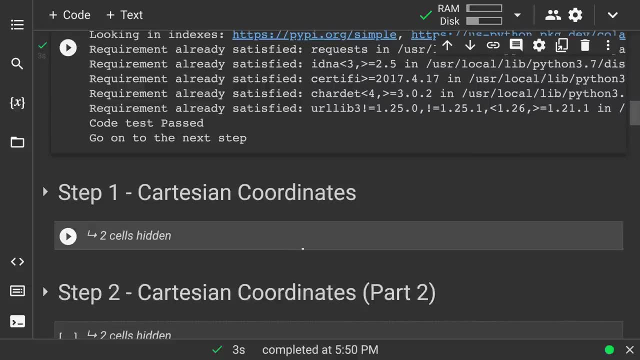 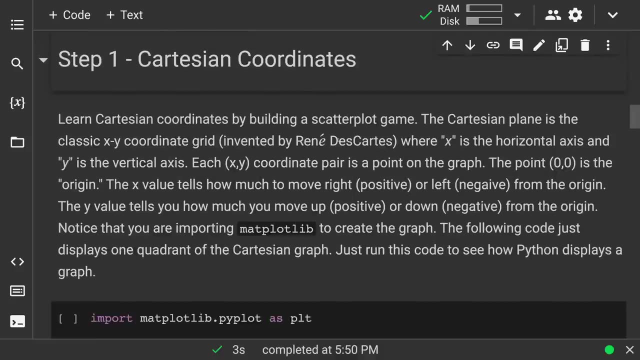 So we click to run Yep And see just a few seconds Code test passed. so there we go. So let's take a look at some coordinates here- Cartesian coordinates, And they're named from Rene Descartes because that's part of his name: Cartes. 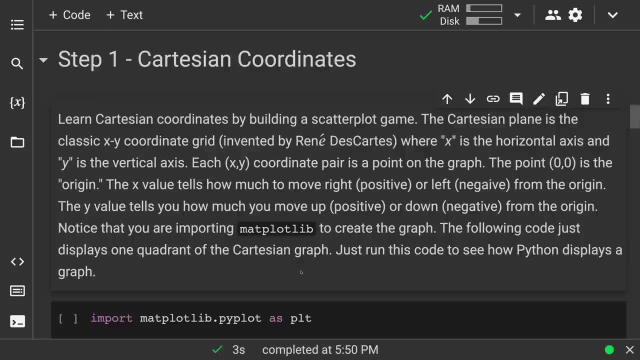 Okay, You know, that's it. You know you've arrived in life when your last name becomes an adjective. So he, among other things, invented this XY coordinate system that we're familiar with, with 00 in the center and then X moving horizontally. 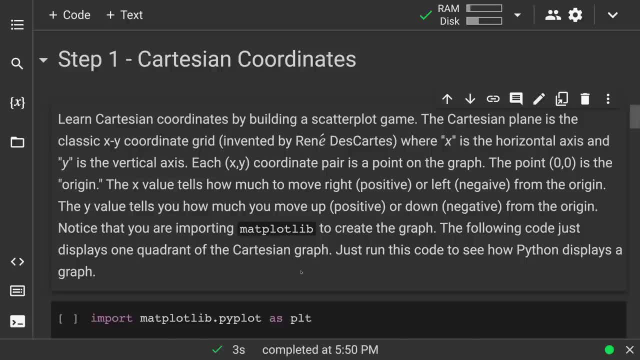 positive to the right, negative to the left. and Y moving vertically, positive up, negative down. So then each XY coordinate tells you, you know how much you're going over and how much you're going up, And we can, we can plot all these points. 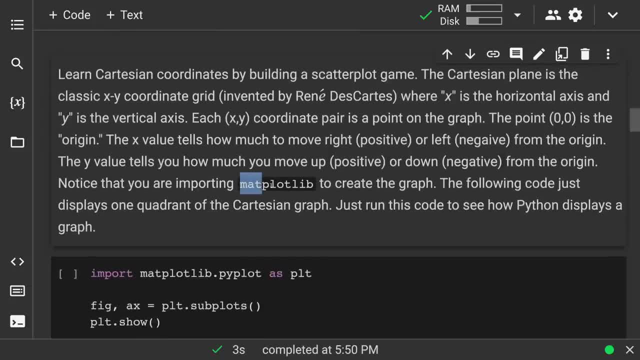 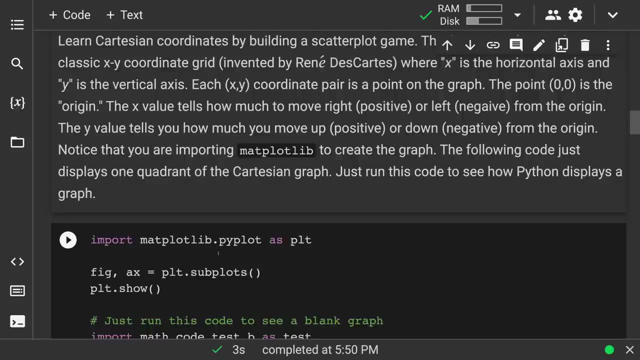 Our go-to library is going to be matplotlibrary And as we were talking about importing your own personal library, custom library, we needed to do that in a little bit different ways. a few more lines, But a lot of the common libraries. 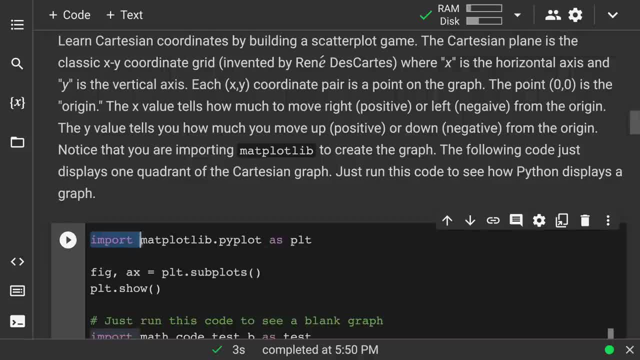 I say common, like you know, reasonably used been around a little bit Behind the scenes. Google Colab already did that install part, So you just need to worry about that. You don't need to worry about importing it. So you know we have that nice benefit. 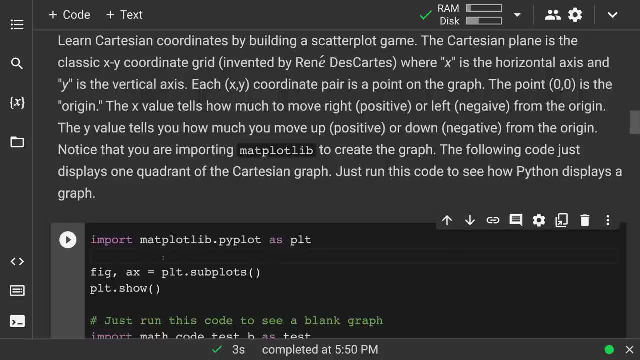 You know, things just work in the Google Colab. So matplotlibpyplot And we're importing this library. Yeah, that's a mouthful. So we're going to import it as PLT That way, every time I reference it. 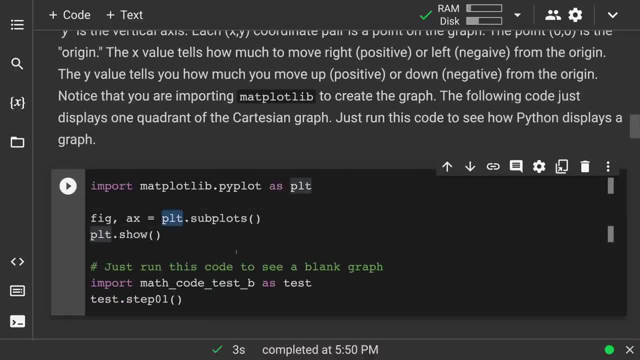 PLT dot. PLT dot. I don't have to rewrite all this. Okay, so this is going to be. the first thing is the basic. just here's a graph. There we go, And you probably could change these variables, but I don't. 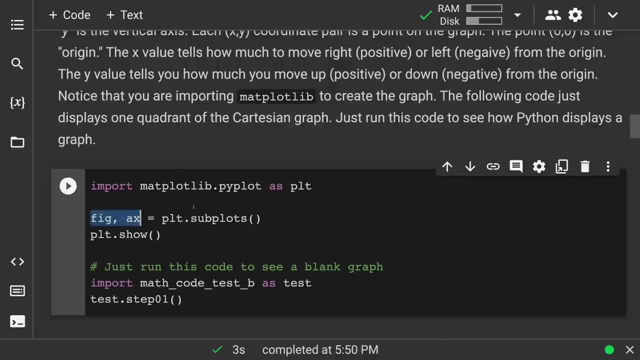 This is what's in the example in the documentation for matplot library, So I keep these, and it does seem weird that you're assigning two different variables to this, but it's you could have multiple subplots. We're not going to worry about that right here. 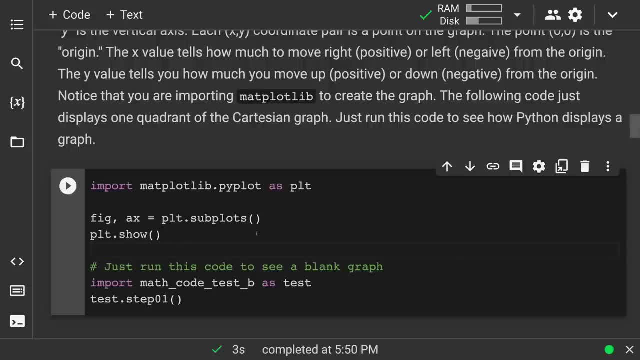 but you could have multiple subplots and you know, your one graph could have like nine little graphs in it if you wanted, or you know, or something like that, but so that you would put numbers in there. but we're not worried about that. 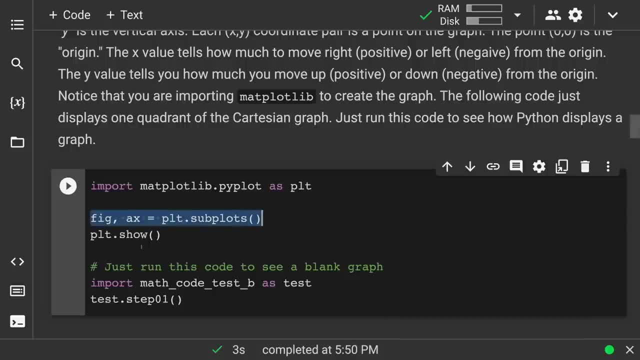 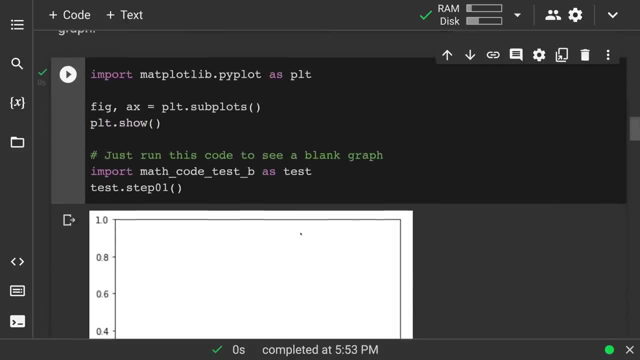 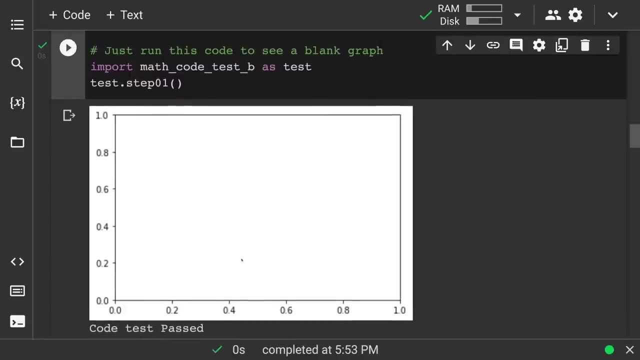 Now, this establishes that this plot exists. and then PLT dot show. That's always going to be our last thing to show it. You run it and there's our basic graph. Notice, we didn't add anything else, So there's not nothing going on here, and zero. zero instead of being 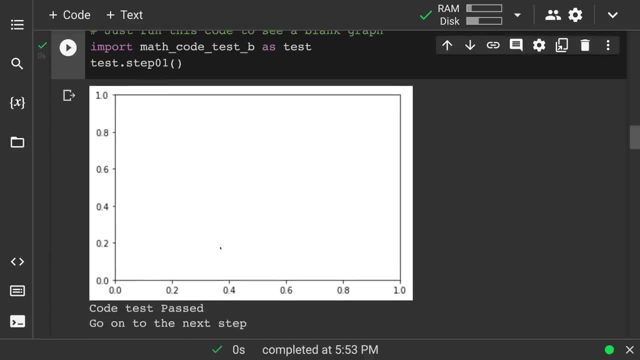 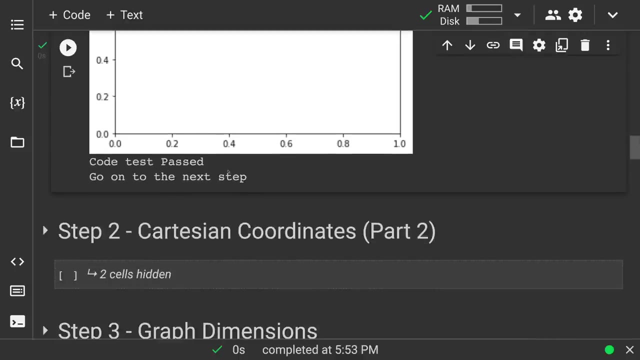 in the middle. it's in the bottom left because we're just showing the positive Quadrant here. So just positive x values up to one, positive y values up to one and that's it. And notice all these, the test and yes code. test passed. 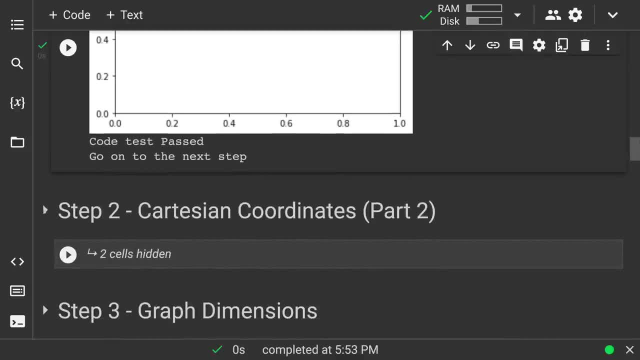 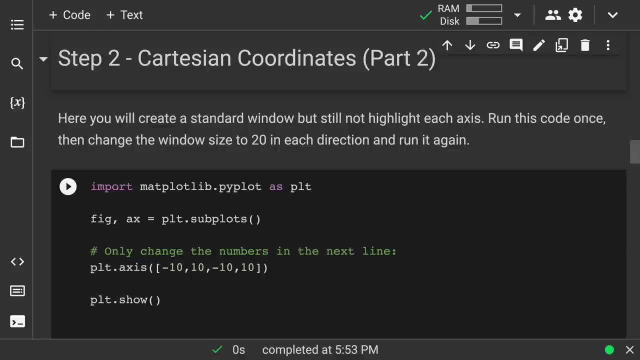 If you click the button correctly, So we'll go to step two. All right, So now we have the standard window still not highlighting each axis, and we're still going to go through import. this establish this. But now we're going to add something here. 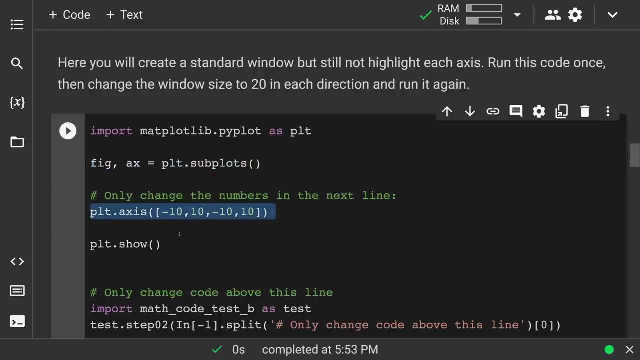 So this gives us the size of the graph, And I just put this here. We're going to this will be better. We're going to modify this as we go on, but that'll give us the size of the graph, 10 in every direction. 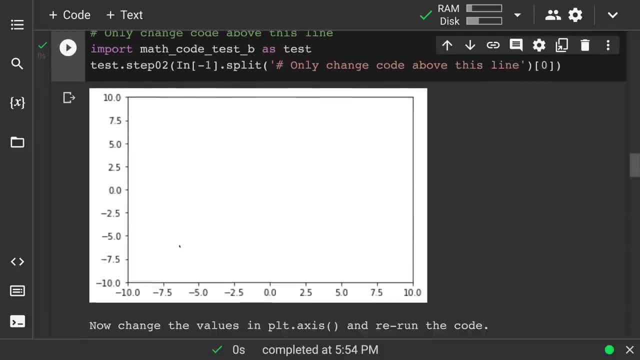 So when we do plot dot show, So you see, it does give us 10 in the direction And if you follow these zero, zero exists in the middle here, even if you don't see the axis lines and zero, you know: positive to the right up to 10, negative to the left down to negative. 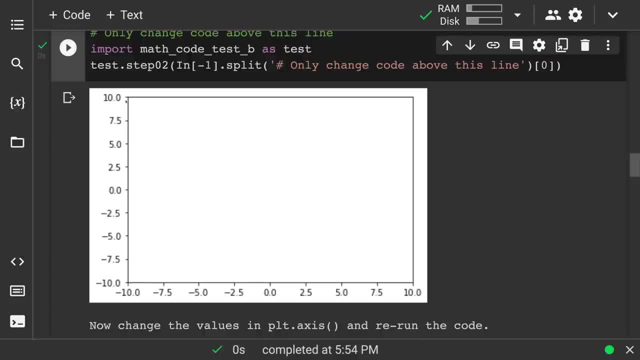 10 and on the y-axis, zero in the middle, positive up to 10, negative down to negative, 10.. So they could line up in the middle here somewhere, All right- and this one was one of these- that I ask you to change the values then. 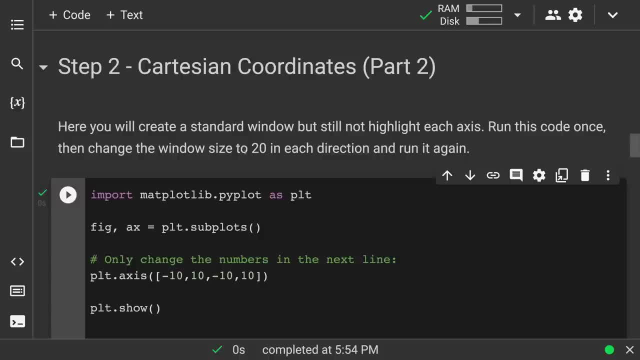 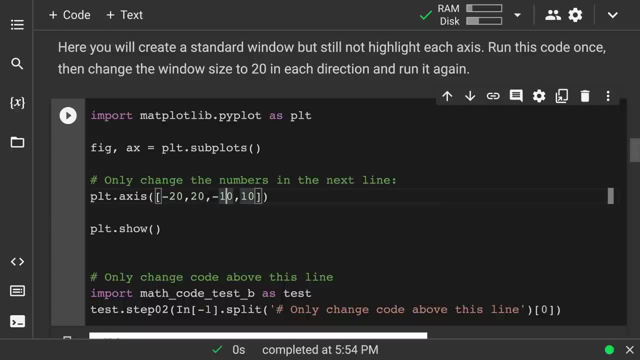 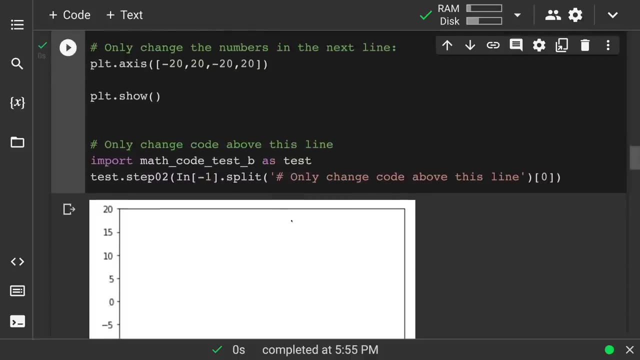 rerun. So it's: run this to see what it looks like, then change the window size to 20. In each direction. So we go through here and we can just move this 20. 20 in each direction. Now we notice from this- even the one where we only went up to one- the size of 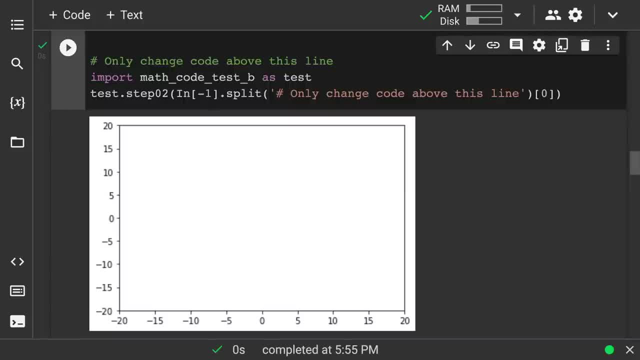 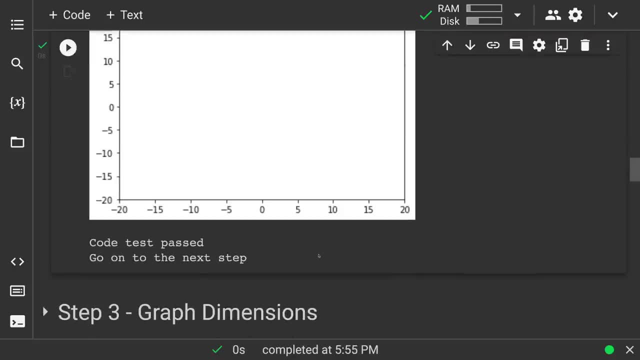 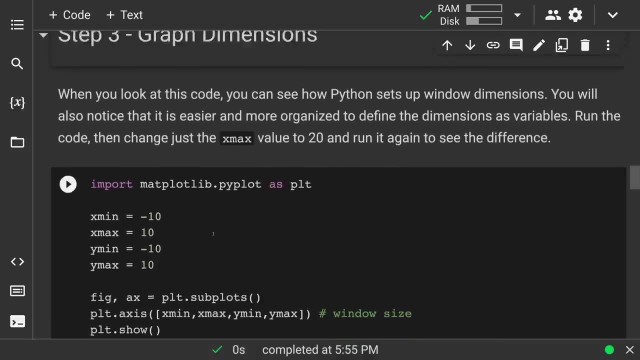 this graph doesn't change, But we see the lines on the outside do and the tick marks change. So now we're going up to 20 instruction. There you go. Code test passed. So some more graph dimensions. Now. this is where I was saying. 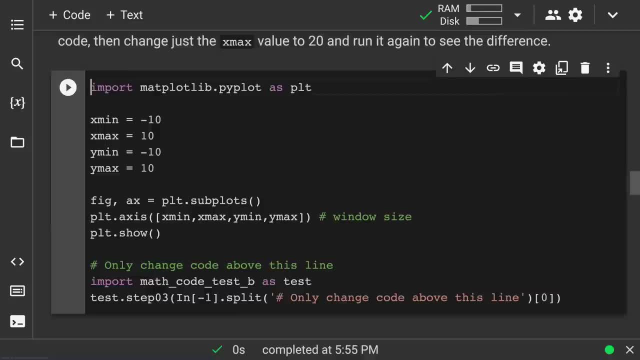 we're going to modify this. This is really what we were doing in that last one PLT dot axis. So what were those numbers? It really was an array of X minimum, X maximum, Y minimum, Y maximum, As just one group. notice the parentheses and then the open brackets. 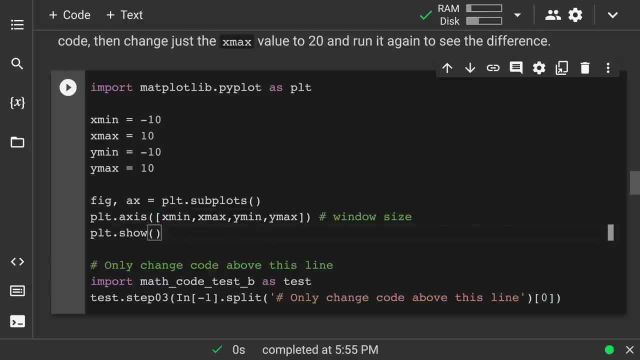 So that was an array and that was that defines the window size. So that's why it's PLT dot axis. So I think it just makes much more sense to define those as variables up here. So this line here, the PLT dot axis, does not need to change. 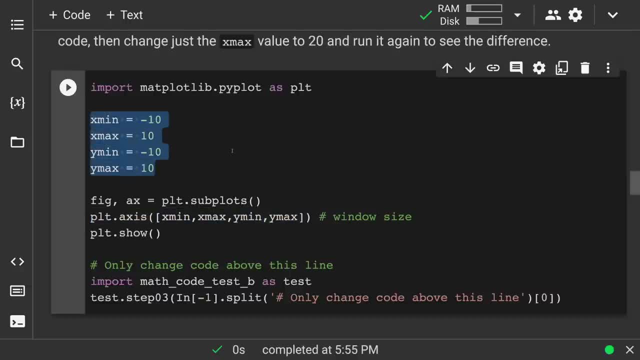 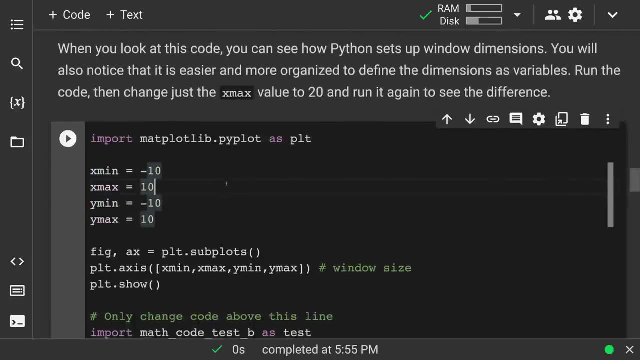 And then it's really easy for you to then change the window size if you want. you just change those numbers. So there we go, And this one is not one I'll show you. this one is: you could run it, Notice it should still do the same thing. 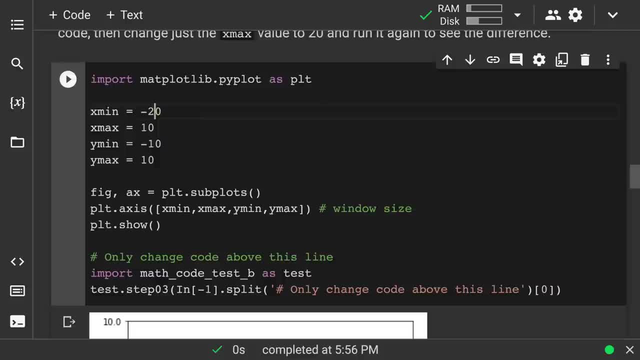 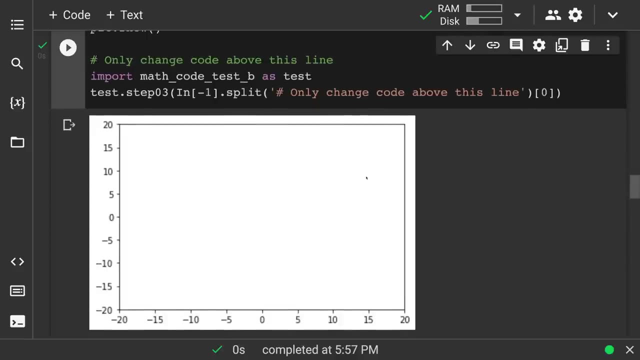 There we go, And then we're just going to change these to 20 in each direction, 20. Yeah, And Again we see 20 in each direction. So This is going to be our go-to Way To set up the graph. 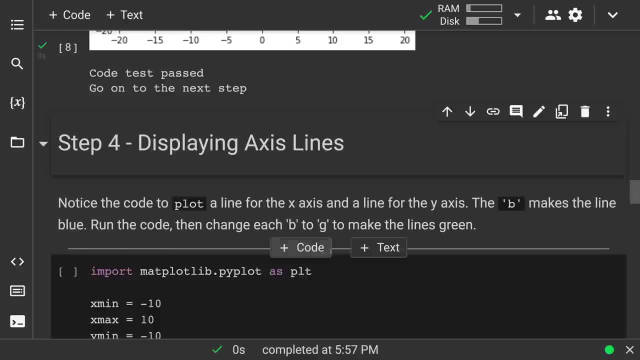 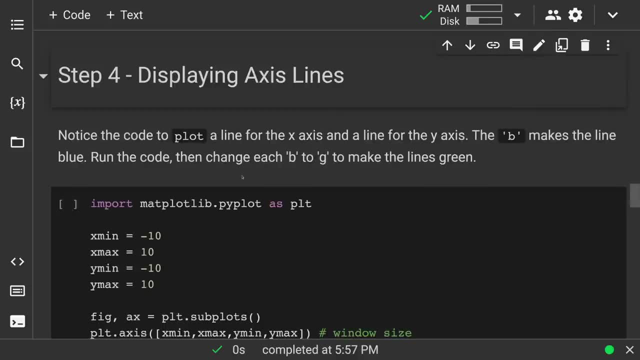 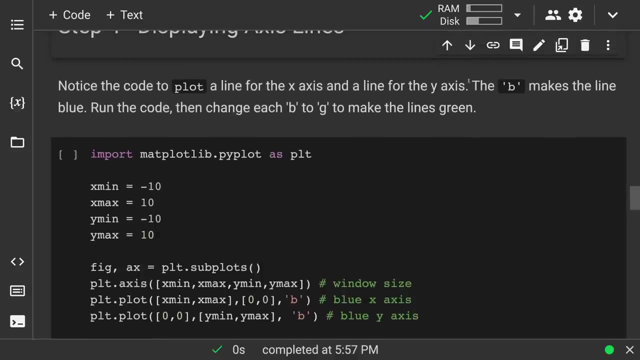 And as we keep going, Let's look at those, just those axis lines that you might be missing. I know I was missing them. So how do we want to display these? Well, We have our basic graph and we have the directions here. 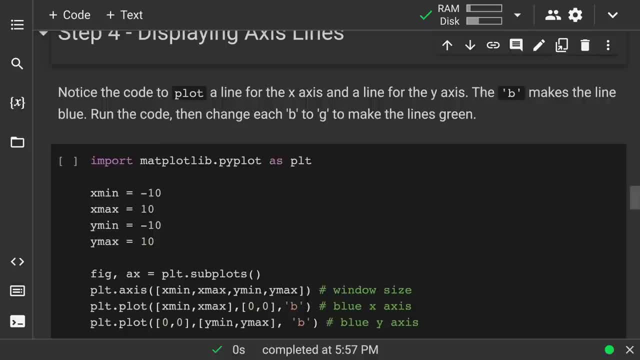 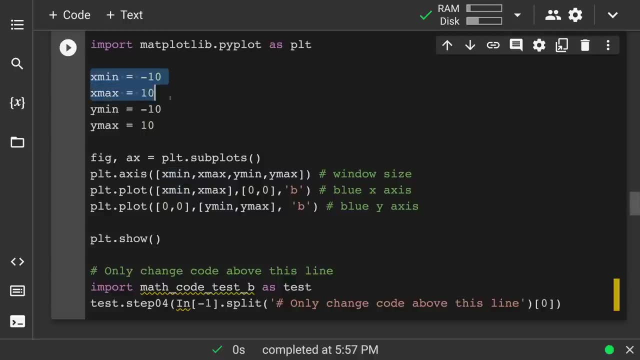 If you were doing this on your own, that the B that we're going to see here makes the line blue. So we have this Dimensions that we were building upon And these first two lines. Rio subplots the window size. So Now we have the PLT dot plot. 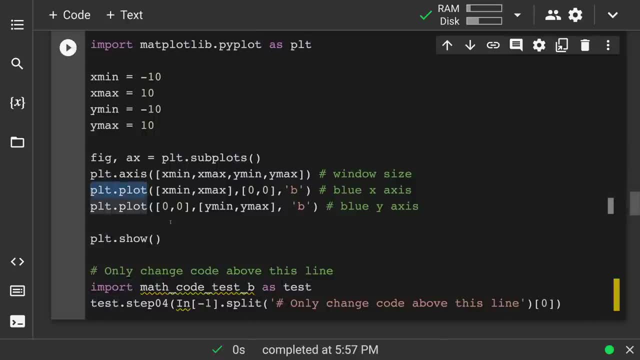 And that's going to get plot a line for us, or points. Now, in this case, we have this array here From X min, X Max, and then this array here. What this is is a An array of the X values and then the Y values. 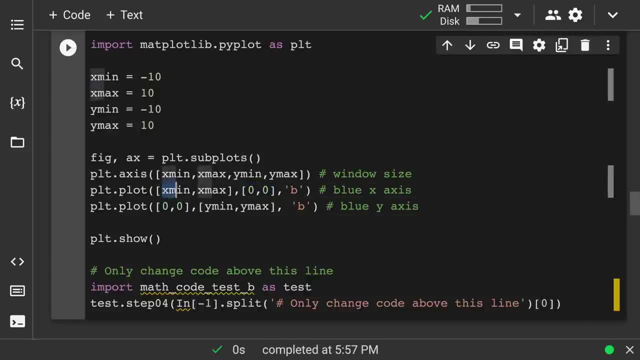 So we have: It starts from X min 0. And then goes to X Max 0. And rather than plot to those two points, it plots a line from that point to that point, And with this the line is going to be blue. 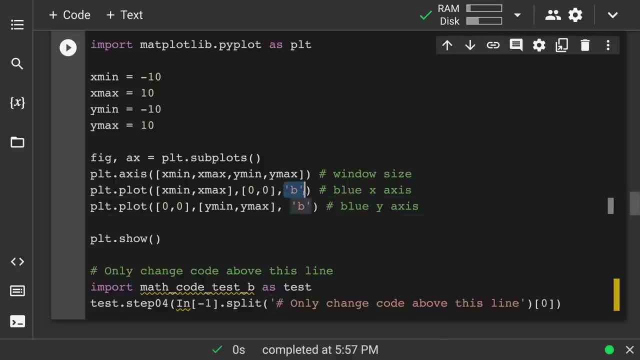 If you don't put something like this in here, Python will pick the color of the line for you And then for the Y axis. Then We're going to plot 0, 0, Y min, Y Max. So what is this telling us? 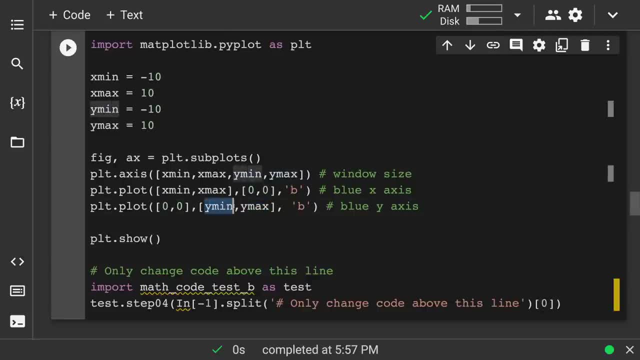 It's from The X value of 0 to the Y value of Y min, So from 0 Y min To 0. Y max. It's going to draw that line And again I'm forcing it into the this, this space here. 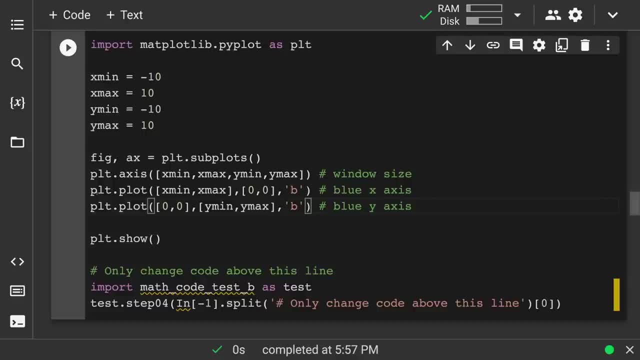 Whether you have the space or not doesn't matter. So there we go. So these two plot statements, These two pull these two plot statements, Define whether you know, define that it's going to be a line, and then what color. and I even have the comments here. 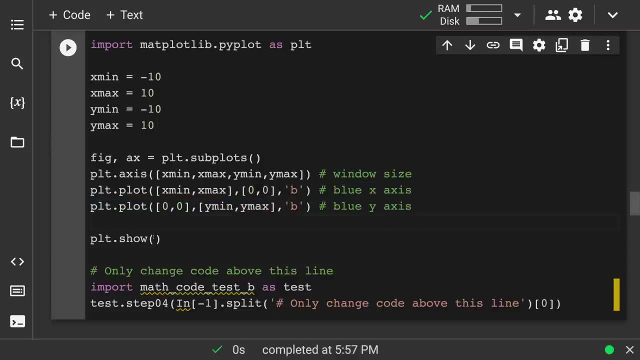 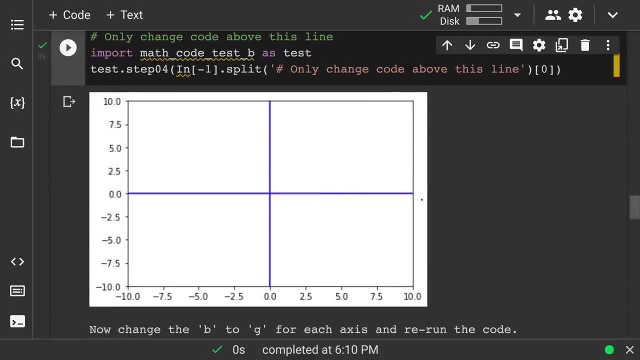 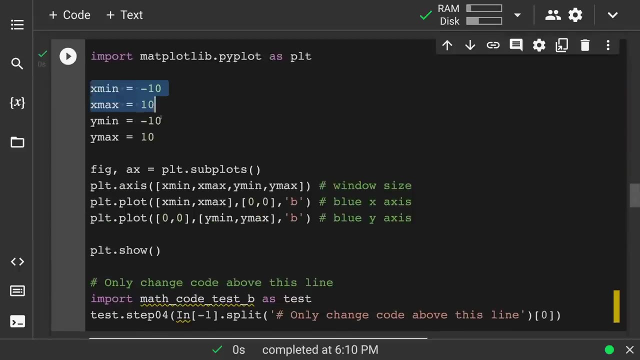 So then you see blue X axis, blue Y axis. So that's it. We're going to show this plot and We see the X and Y axis. We also see again the value of defining everything up here, because then all the rest of these 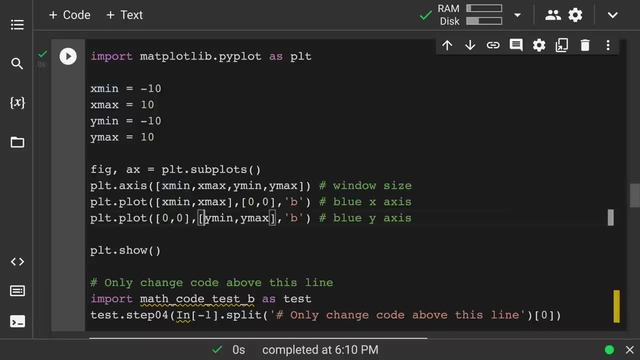 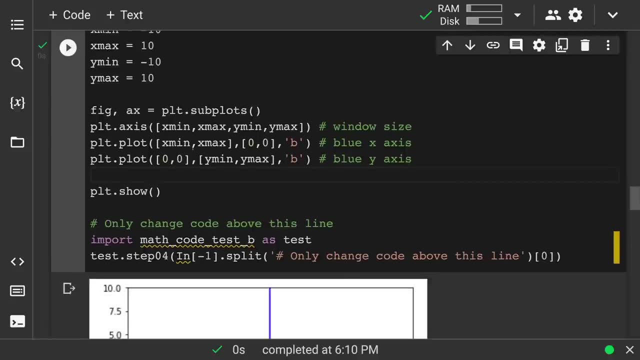 The size of the graph and then where these lines go To and from. It's all based on this up top. So if I change the dimensions of this, Then everything else will just accordingly. in the axis lines will still go to the end. 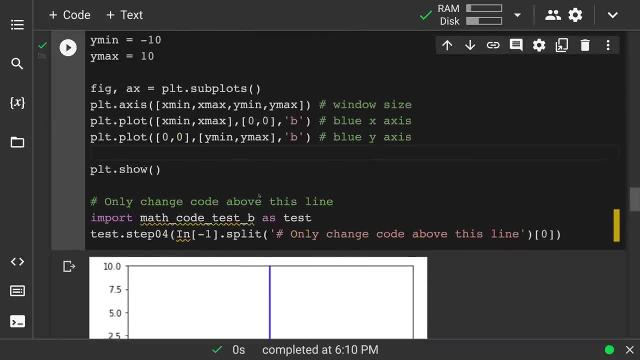 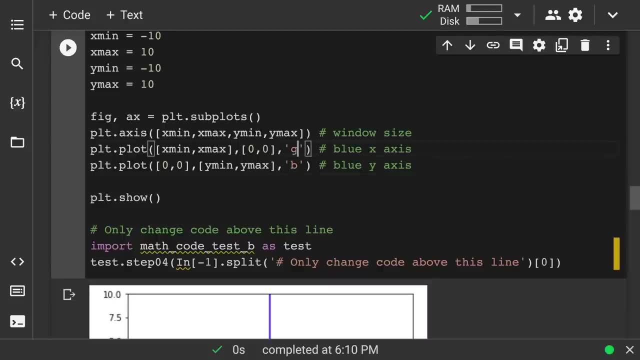 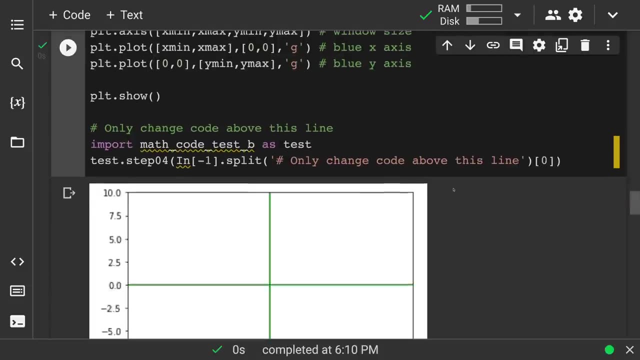 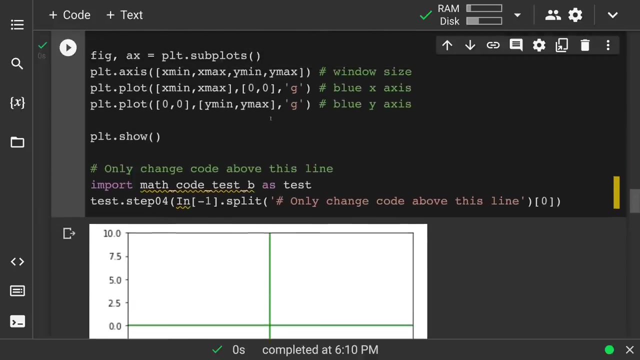 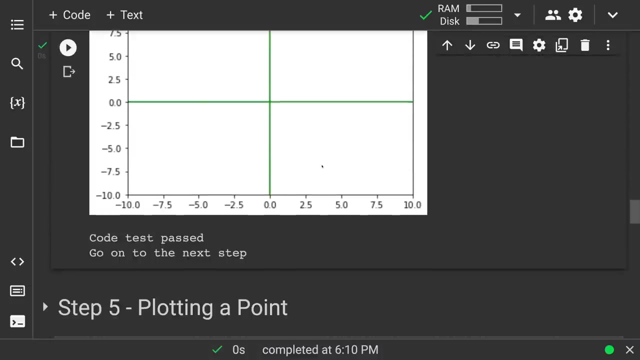 So we run it and then change B to G, And We go change to G, And there we go. It's green, So You can make it whatever you want. I just happen to like blue, So there we go, Changing these. 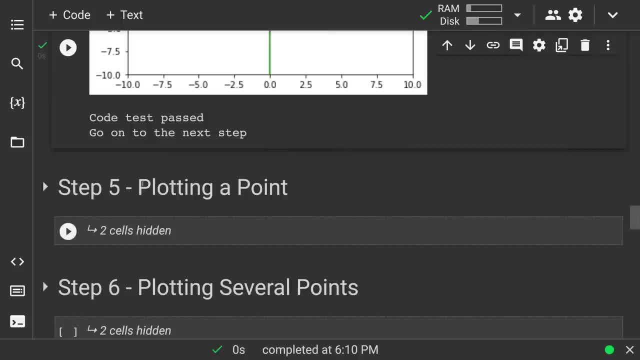 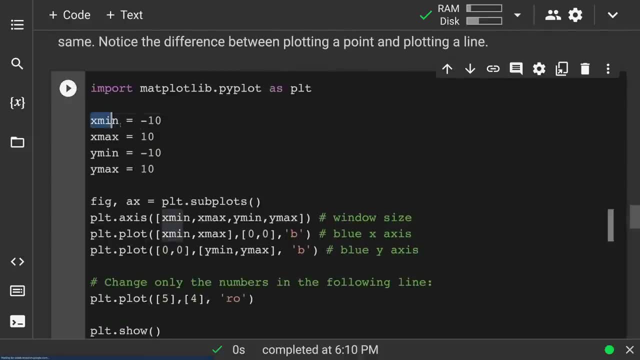 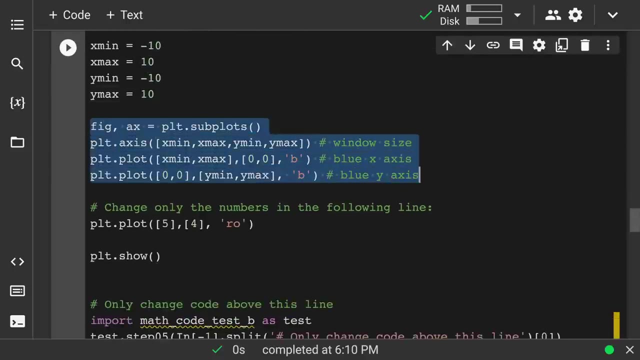 So now, supposing I want to plot a point, like we saw that we did that into define a line. We're going to plot a point. Well, See, as we continue to build this, define these values here, and now we're going to, we're just going to end up keeping all of this. 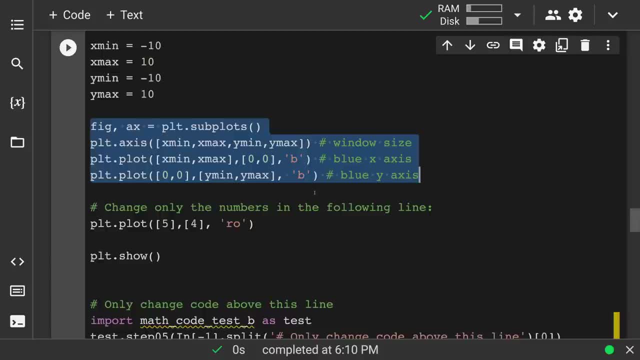 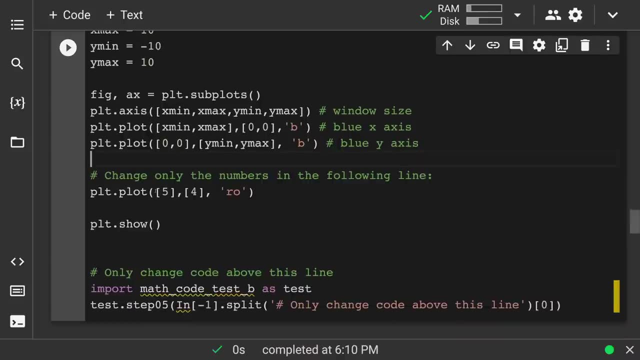 As the window size, and then the X and Y axis And keeping it blue. So how do I plot exactly one point? So notice this array of X values, of which there's only one in there, and Y values, So it's five, four. 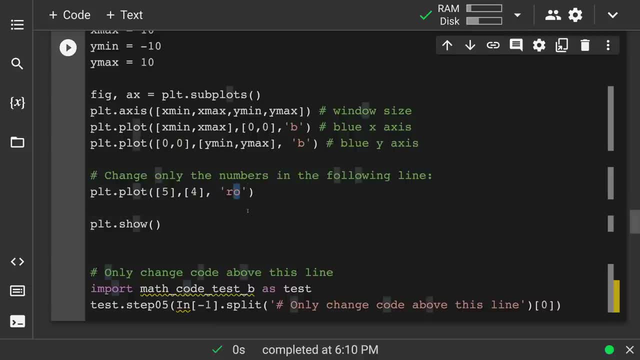 Now here's what else we have. It's our oh. that oh makes it a point. In fact, a circular Dot. So if I have just be with nothing, that's going to make it a line. If I actually just had our with nothing, that would make it a line. 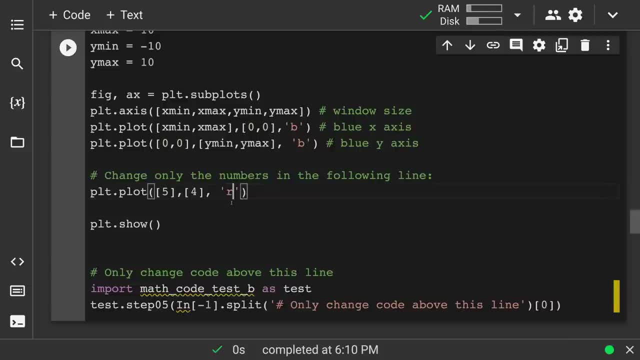 But it actually has nowhere to go to. So that would be weird. But our oh makes it a point And we'll see we can Plot other things too. So keeping all that the same and just plotting this one point, There we go. 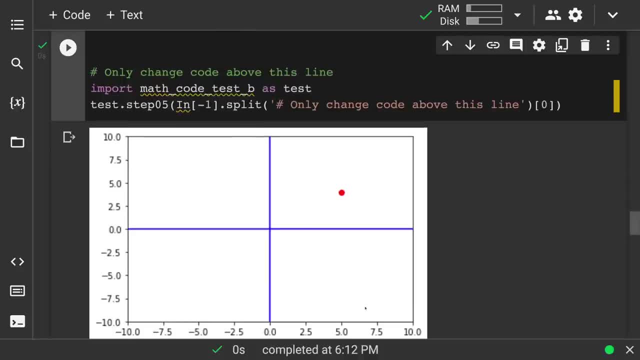 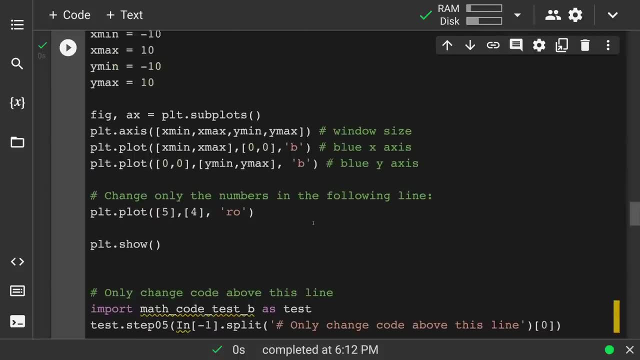 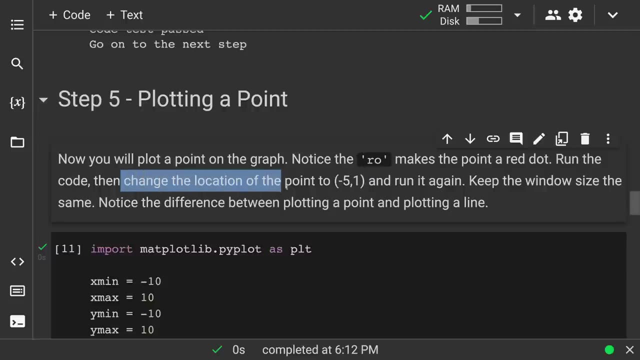 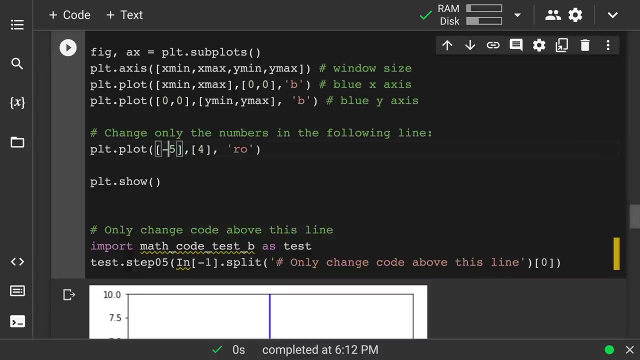 One point, and it is five at five, four over five up, for We could put the grid lines in, but that'll be another story. So now change the location, So the directions run it. then change location to negative five one. Okay, so then we just change this to negative five. 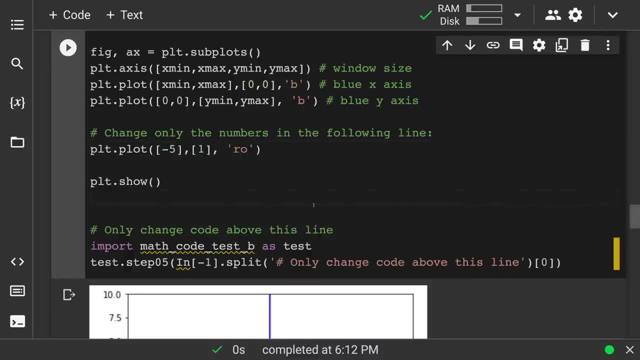 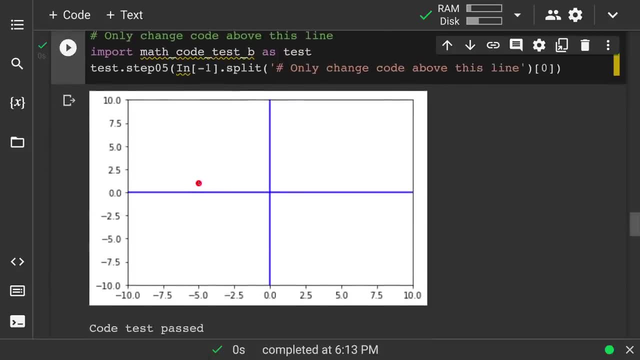 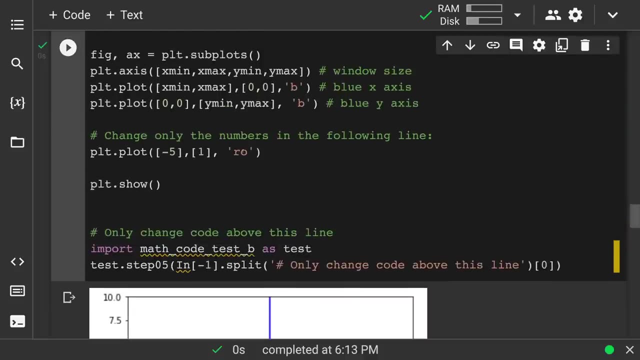 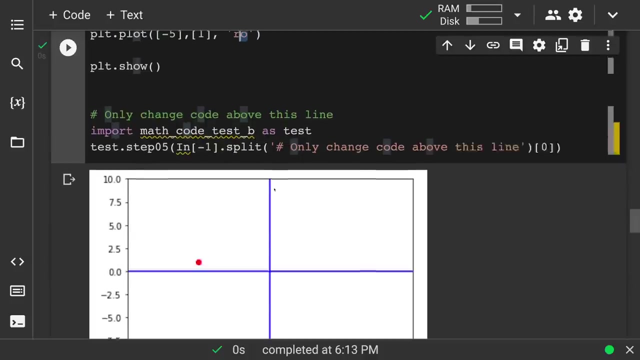 And change this to one. There we go, And when we run it So we see negative five one. All right. So plotting a point, We indicate that it's a point this way, and Plotting a line, We have other ways to indicate that. 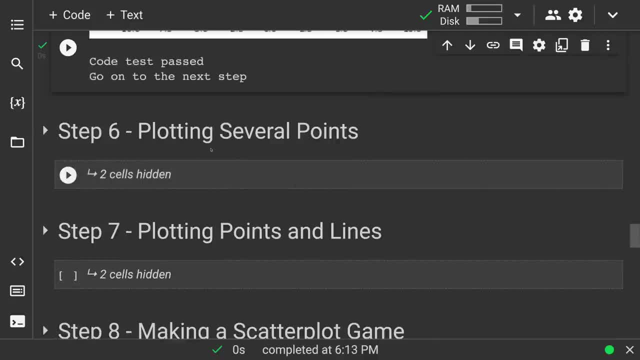 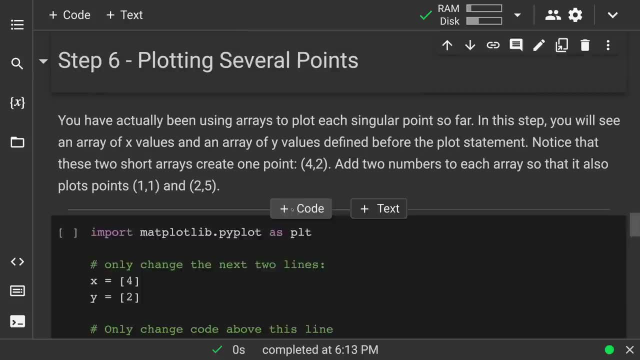 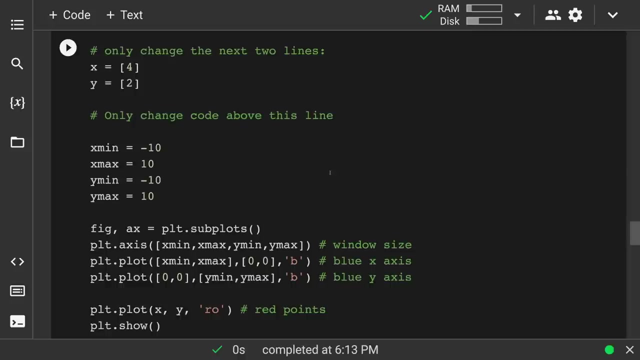 So how would I plot several points? Well, let's take a look. All right, so Arrays to plot each point. You know, that's what we've been doing And We can still define it as an array here. I'm just going to define the array here: an array of x values and an array of y values. 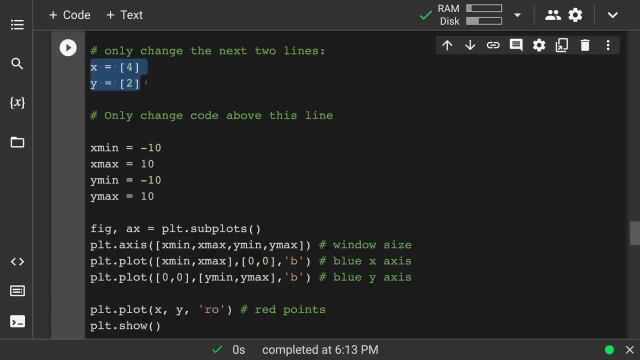 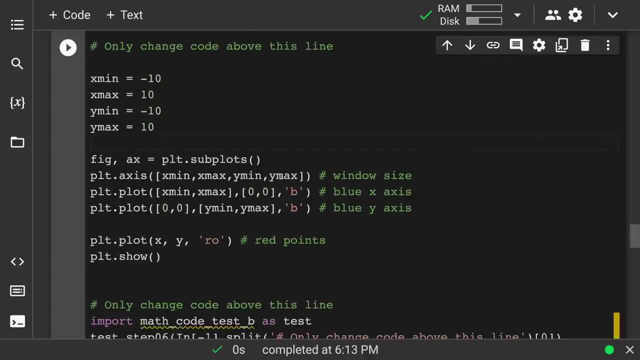 So If I have these x values and y values, We go down here. So notice, all that's still the same. and here I can plot xy Now. I chose xy because you know x values and y values and I did not use exactly x and y as other variables already. 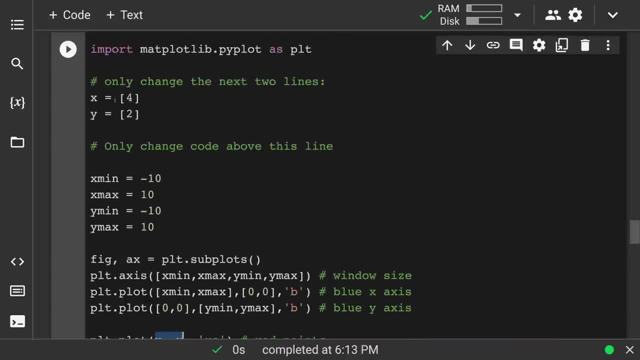 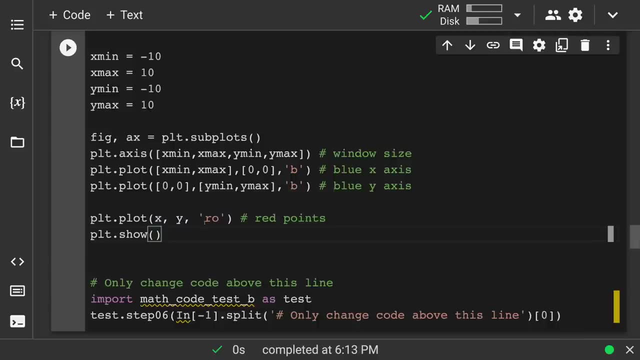 So we're okay. I mean, you really could name these arrays whatever you want. But there we go, We have what am I plotting? the array of x values, the array of y values, and then Here I have Red points for each of them. 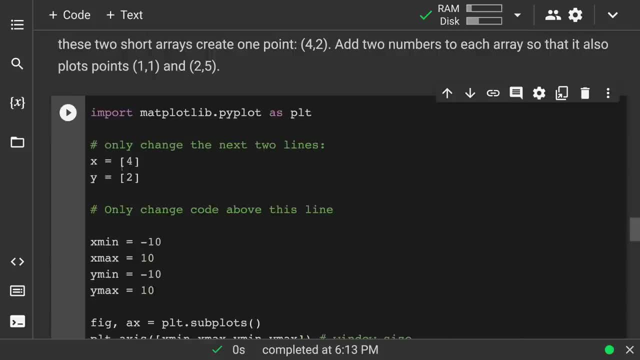 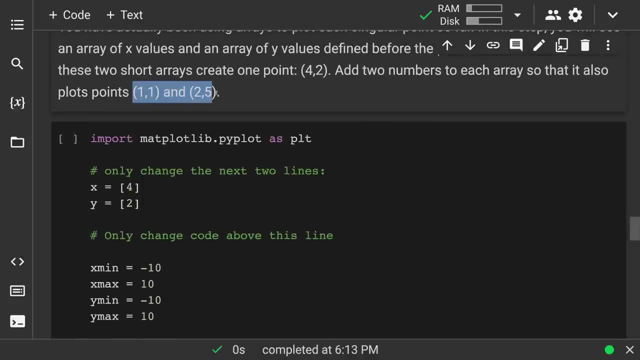 Now, right here I only have one l, one number in each so we can add. so that's the assignment for this step. Add two numbers to each, so that also graphs: one, one and two, five. Okay, So the x value would be one. 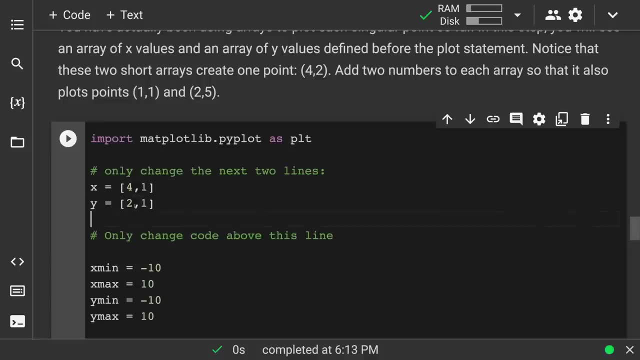 And the y value be one. So there you go. So I have Point four, two, and then point one, one, and the next one to five. So X value would be two, Y value would be five, And there we go, All right, and 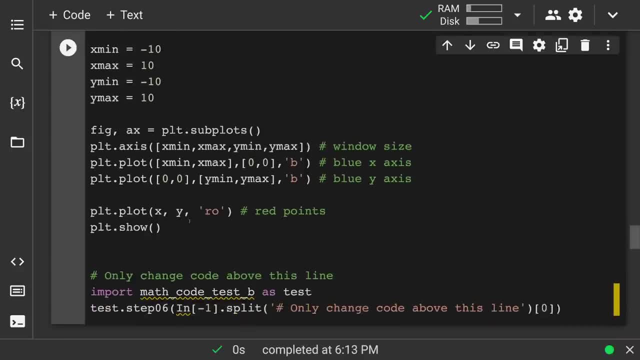 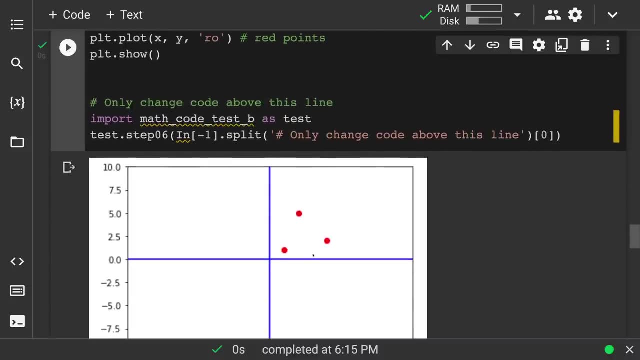 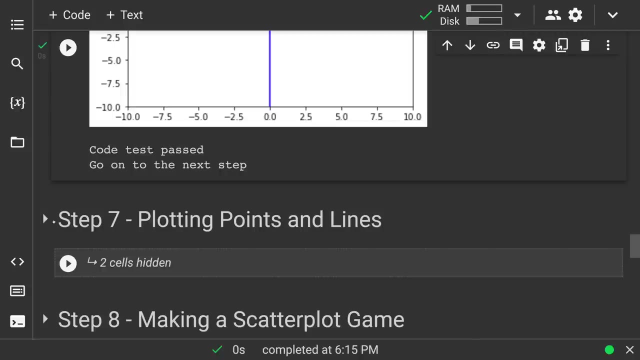 Changing those arrays. Now I can plot- I still don't Have to change this code- plot that array And we see three different points, Because each of them I made A red point. So let's mix it up. Let's plot some points in some lines. 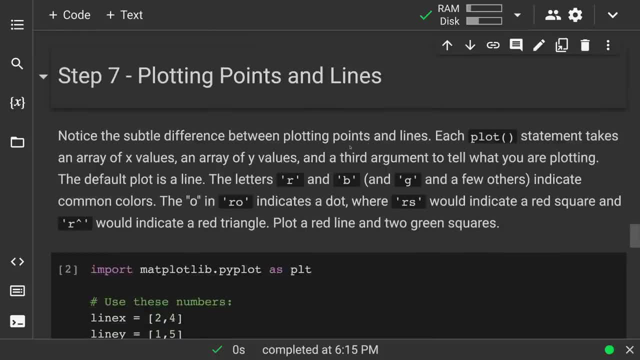 Okay, so that's it. Hopefully you are noticing the subtle difference between the points in the lines. Each plot statements takes an array of x values and array of y values and the third argument to tell you what you're plotting. So the default plot is a line. 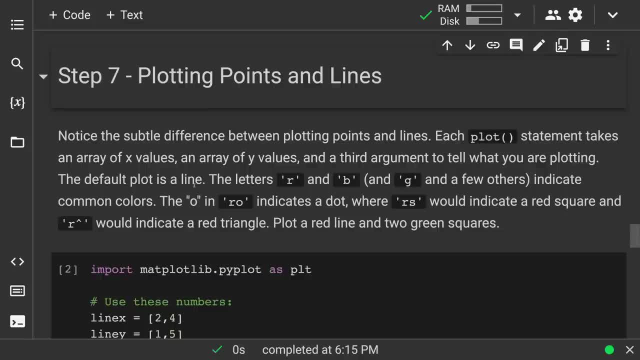 If you actually skip that third argument, it would give you a line and Python would pick the color. RBG indicate the colors, and CMYK actually also work as just letters, And beyond that there's actually a few other colors where you can just write in the word for the color. 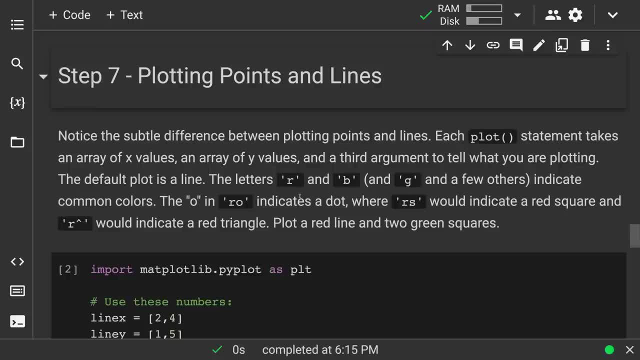 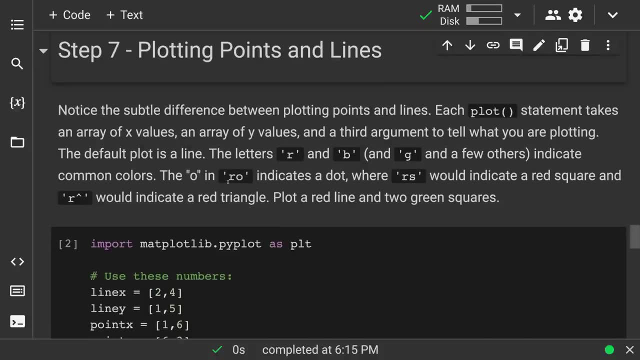 Give it a try. You know I'm not going to list all the possible colors, but yeah, give it a try. And so these are the colors. So then we have. if it's a dot, it's going to be RO. 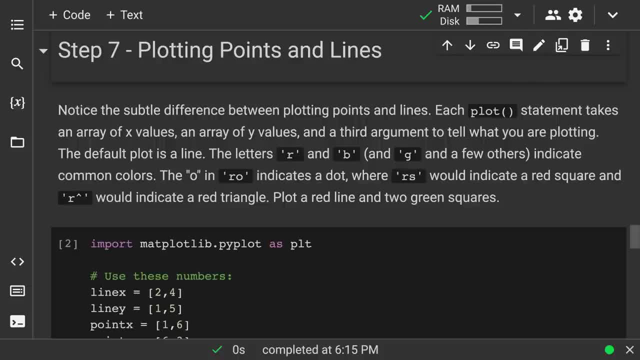 The O indicates a dot, RS. You could plot a square And then R with a little carrot symbol would be a triangle, So that if you have different things you're plotting, you can mix it up and have dots or squares or triangles. 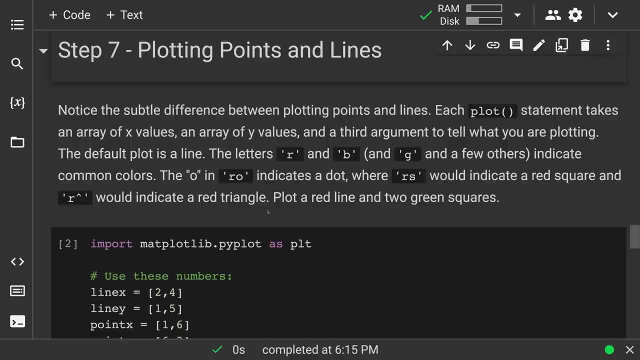 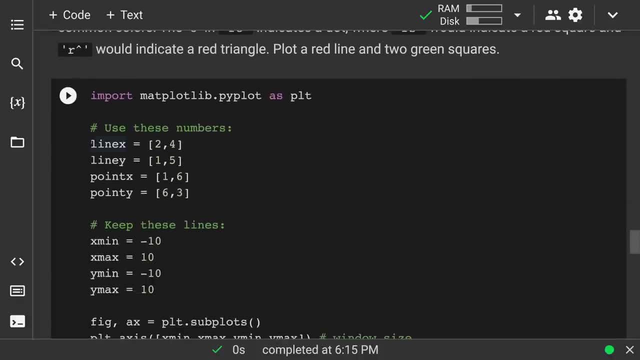 And then, of course, that, combined with the different colors, you can plot a lot of different things on one graph. So notice, we've already defined these arrays here And I'll call this one: line X, line Y, point X, point Y. 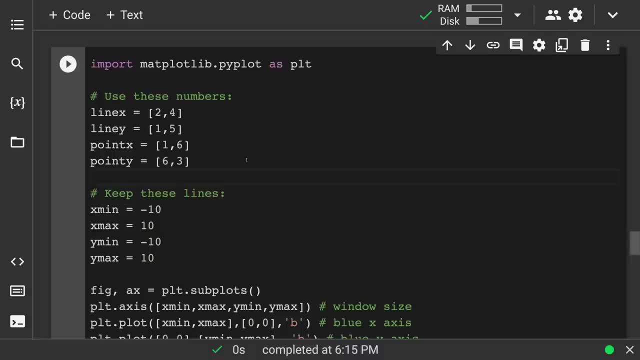 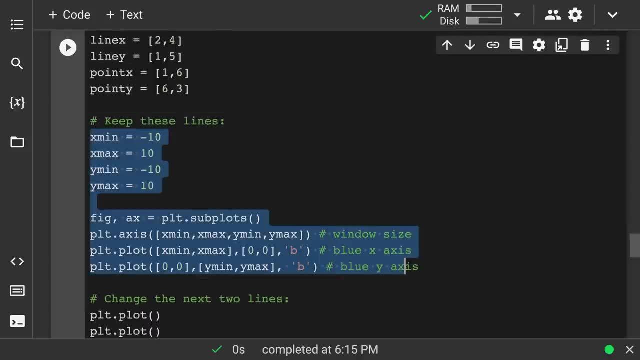 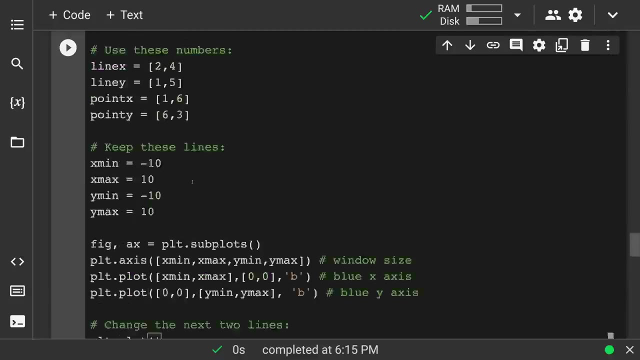 So yeah, not liney and pointy. And there we go. So we have these. We'll keep all these defining the graph the same way And let's plot. So if I wanted to plot. So the directions are: Plot a red line and two green squares. 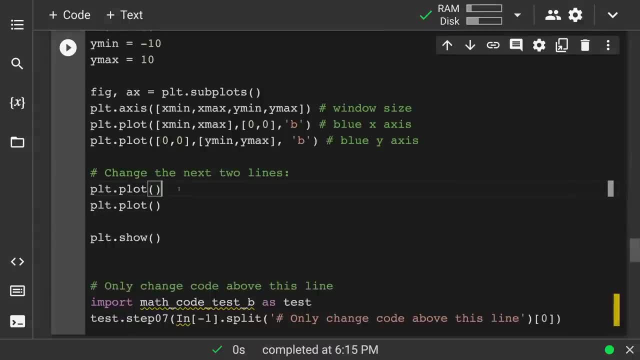 So if I plot here, So line X, line Y, and we want it to be red, and it's a line, So there we go, And point X, point Y, and it's a green square GS. So you see if you've been working through the course, hopefully this is a review. 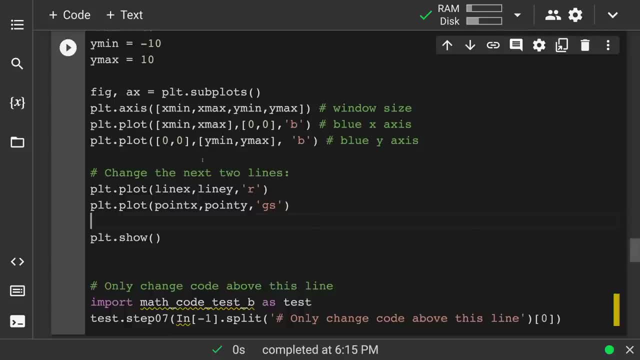 And if you're coming at this, you know relatively new, hopefully it's seeming pretty straightforward, But then the more you do this, the more You just get familiar with, with graphing everything, and you know be able to do this right off the top of your head. 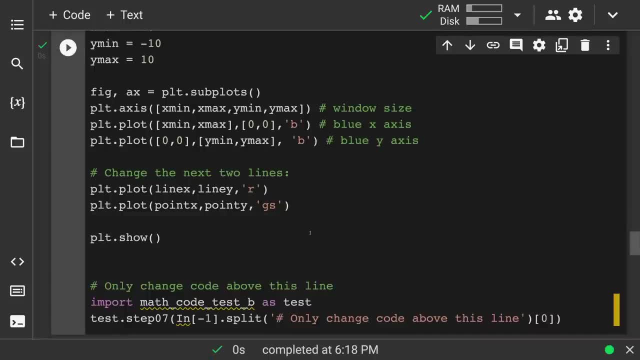 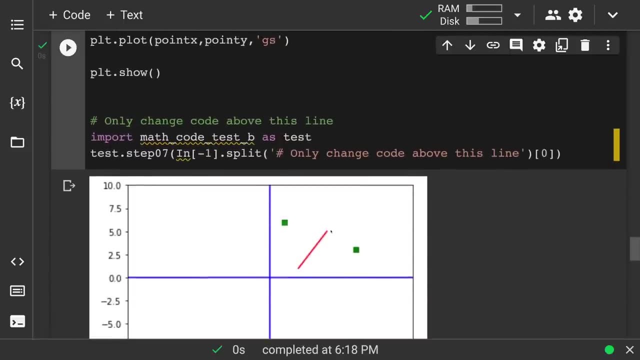 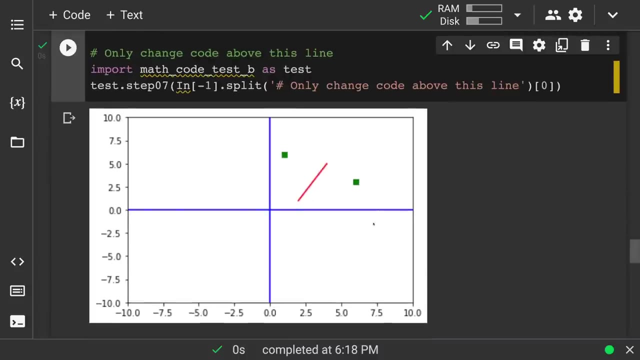 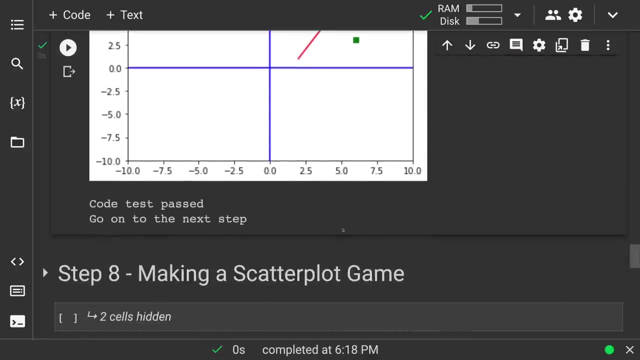 So we graph this And we will see. So there's the red line from that point to that point and the green squares over here. So there we go, So we see how we can graph a line And different points. Okay, so here's a scatter plot game. 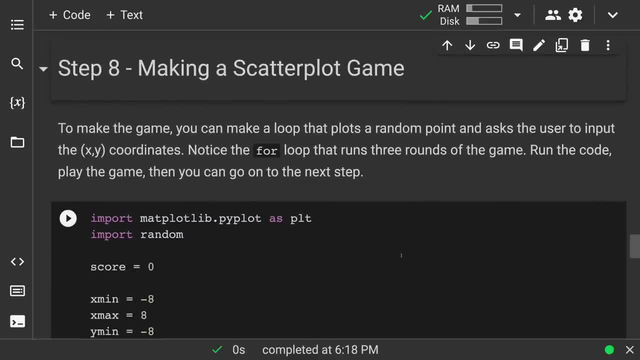 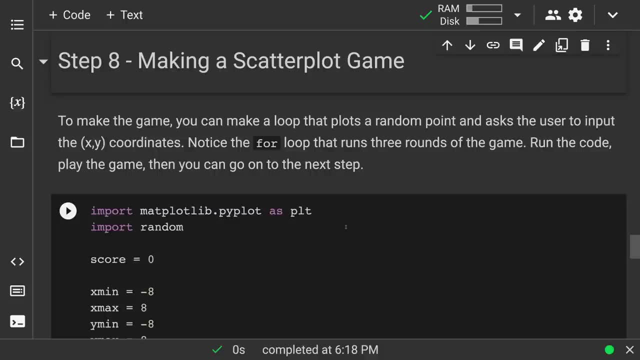 And I call this making a scatter plot game, But I kind of made the game so, But we could take a look. So this is what we want to do. We want to look through this code. How can I plot a random point? 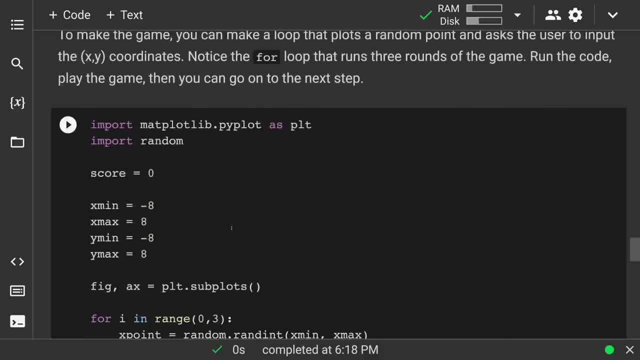 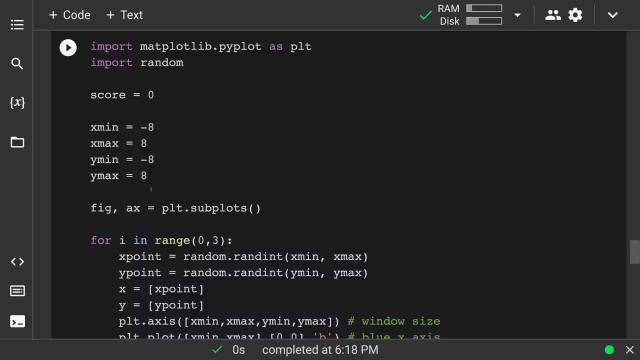 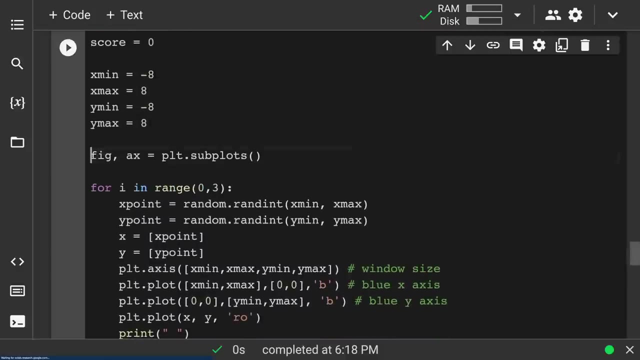 And then you know, you're going to try to guess the point. I made the. I made this, you know, a smaller axis, for whatever reason, And We'll define this once. And here's what we're doing each time. 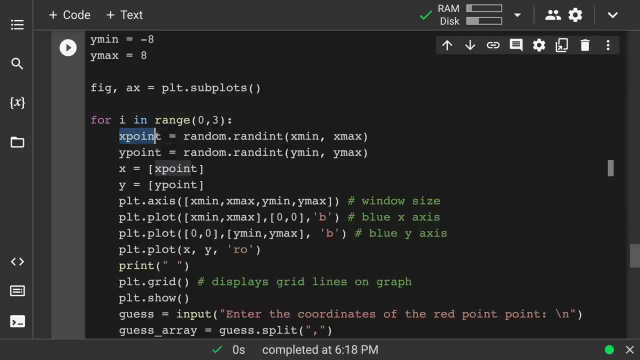 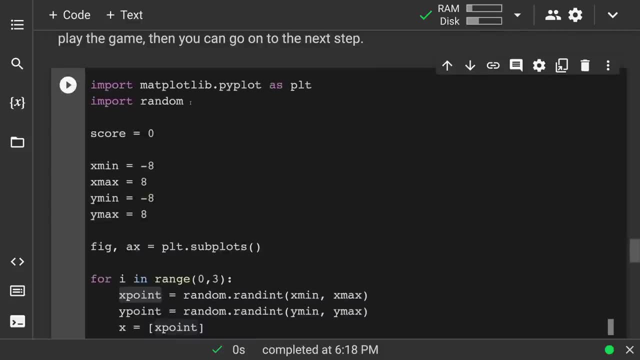 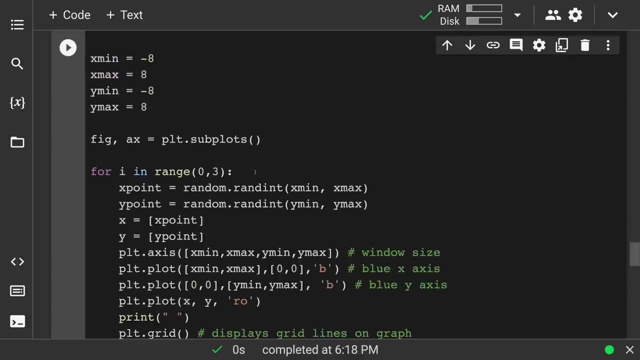 If we are, We're going to get an X point, which is going to be a random number. So notice how this, this is going to be good for different games or different things. You do Import random. Yes, there's a whole library of randomness. 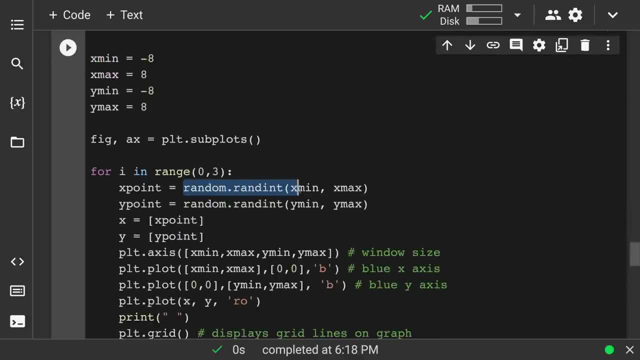 And random dot rand int And it gives the range here From X min to X max. and actually the way most ranges work in Python. X min is a possibility but X max Is X max. It will. won't go to that. 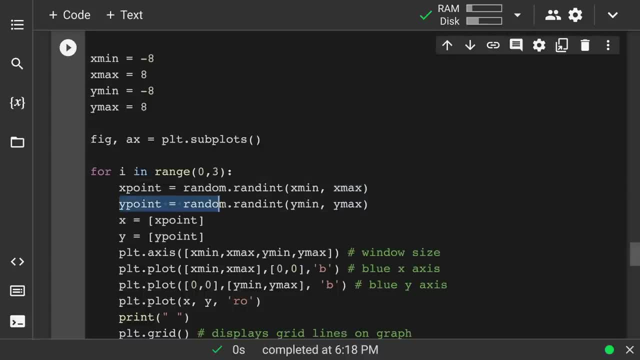 It'll go to the number before. So why point Y min, Y max? So there we go. So you see again, if I change these dimensions, It will still give me a random integer that's within that. So Now, if 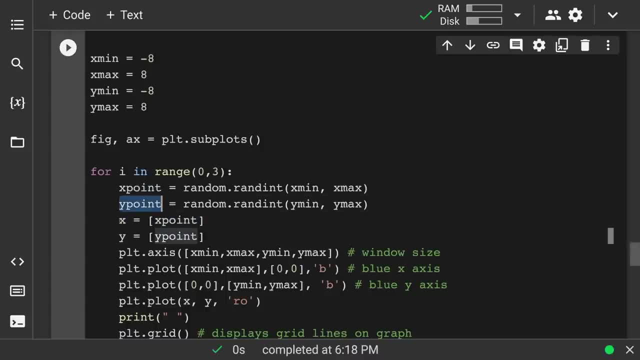 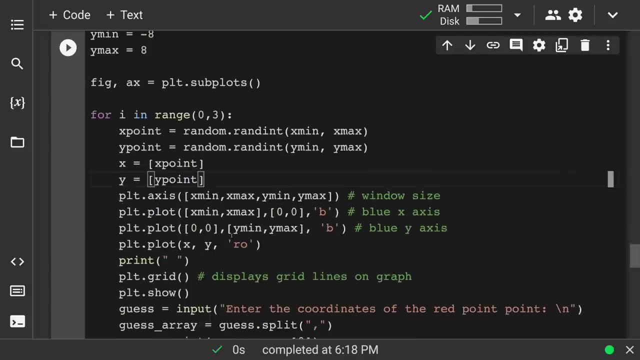 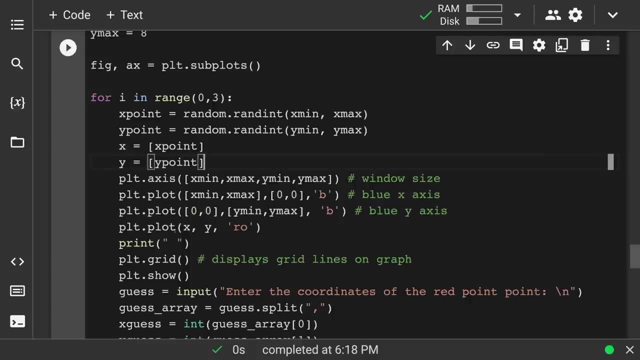 X point is the random integer, Then I'm going to store that as my X value Store. This is my Y value And you see, essentially it is an array with one element, You know. But then And I 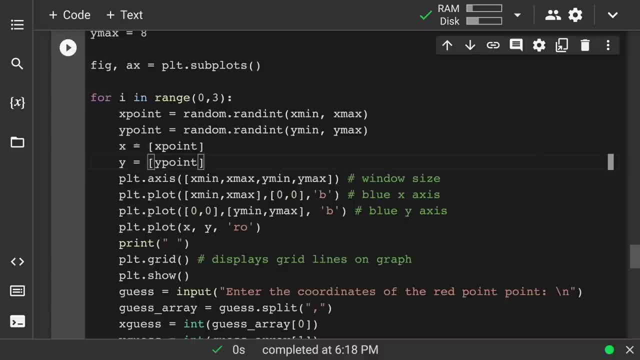 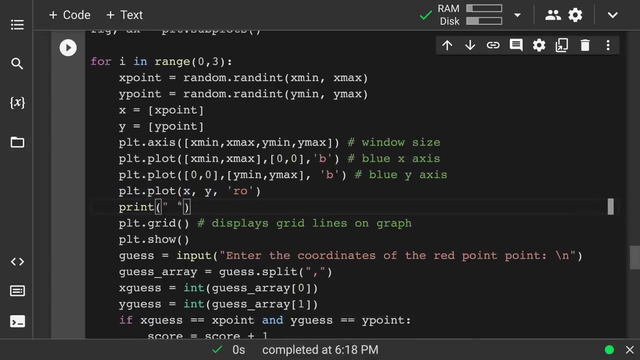 Might have been able to skip this step, But I like really spelling it out. You know what this is And now we go here, I'm going to apply As a dot. So there we go. This gives the grid. Now, this is we. you know, we had their access lines. 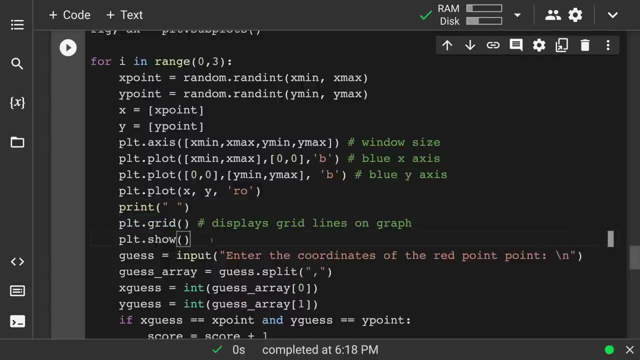 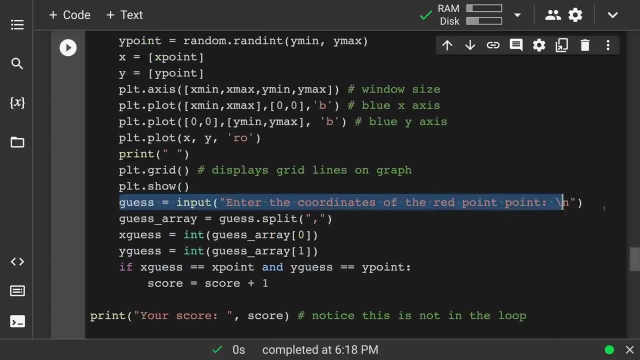 This is the grid: PLT dot grid. So That'll help because the game Is going to be. here's the point. You tell me what The coordinates are, So That's what this is. Yes, And we're going to prompt for input. enter the coordinates of the red point. 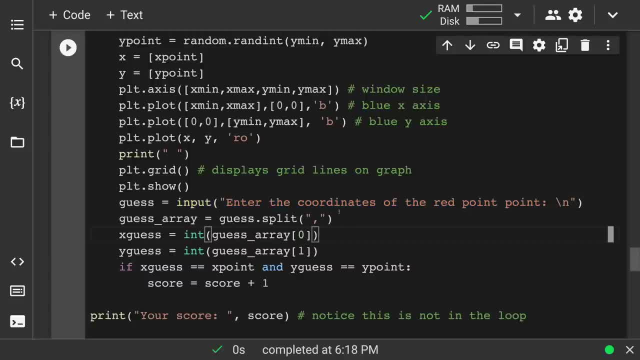 And that's going to be an XY with a comma, So We're going to split it at the comma And that's going to be an array with two elements. So then, Yes, Array zero, So the first element cast as an integer. 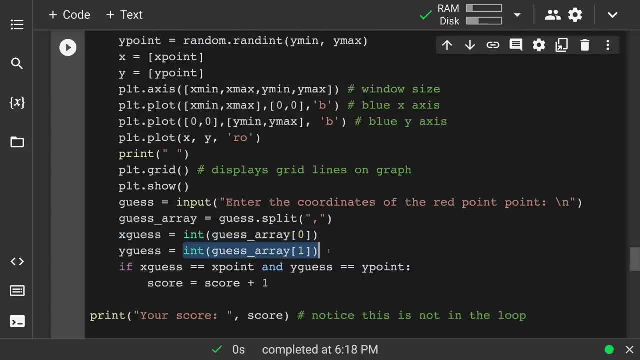 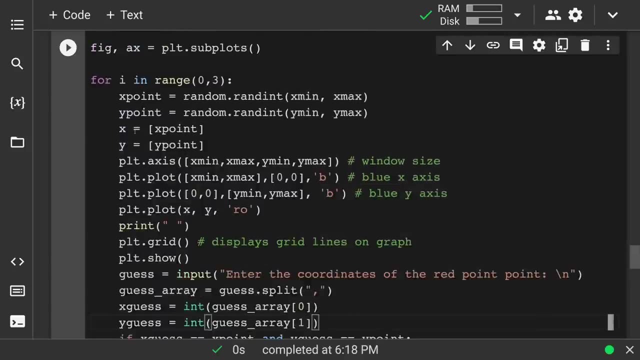 That's going to be the X gas, And the second element is the Y value cast as an integer, That's going to be the Y gas. And this is part of why I like to break it up here, Because I have this here. 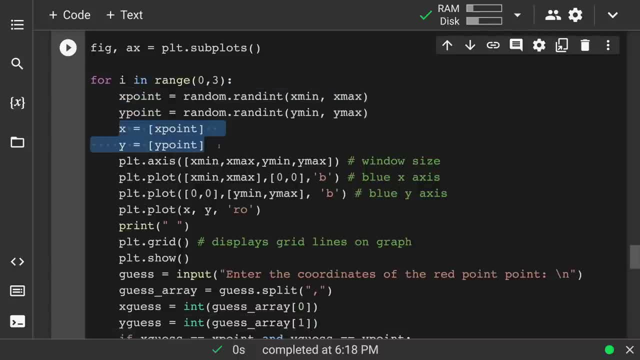 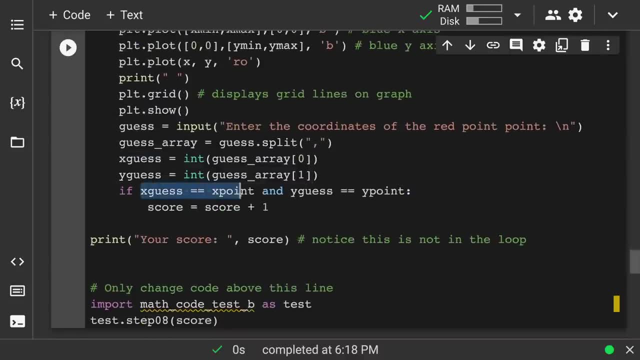 These are the points. This defines it as an array, But this is the point that we wanted, So we test it. if X guess equals X point, And why guess equals Y point, then that's going to increment your score. And there we go, all this in the loop. and then, if statements in the loop 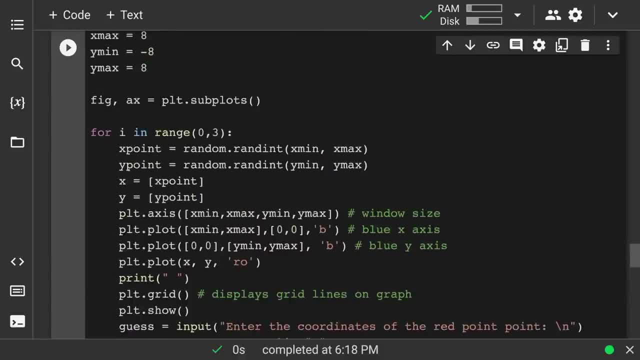 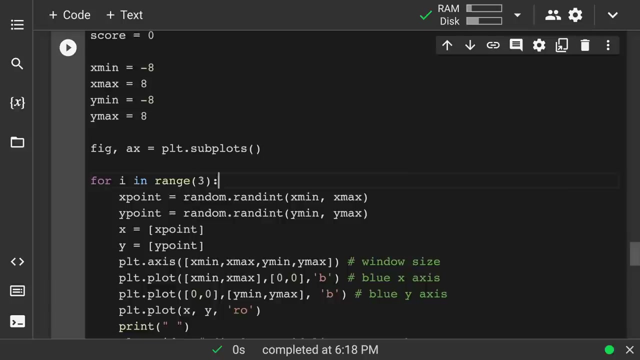 Now the loops done and You know, in range zero to three, we really, because we're including zero, We actually don't need that zero- The range will start at zero by default. So There you go, for I in range, It's going to go through it three times because it'll be zero: one, two and then again Python ranges. 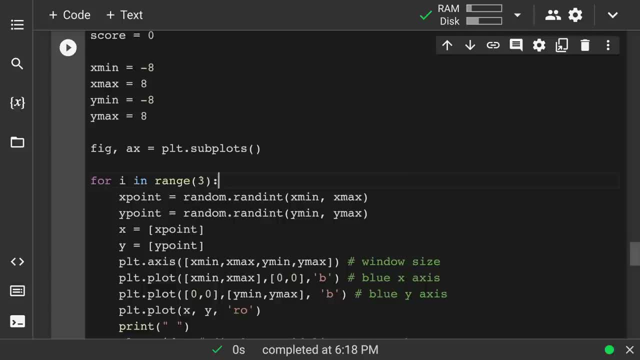 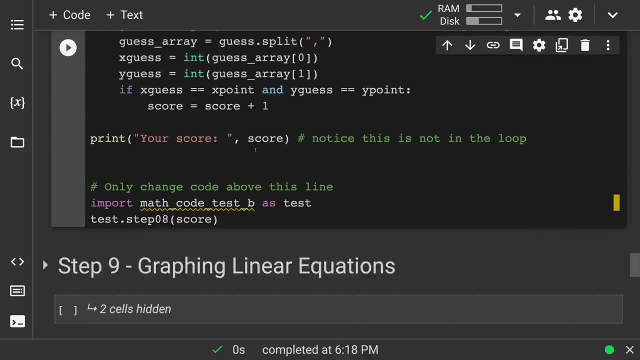 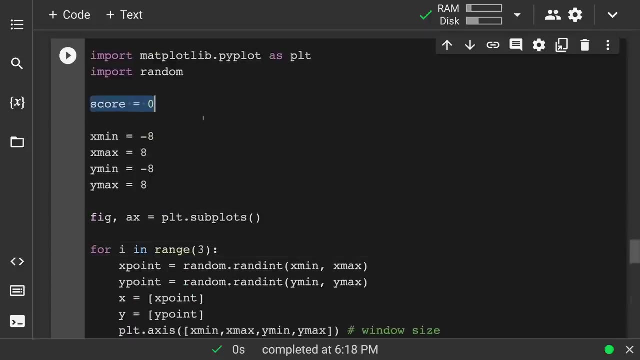 If it's range three, it won't do three. it'll do zero, one, two And then that's it. So We go through and guess it three times and then Print out the score. So the score Was way at the top. 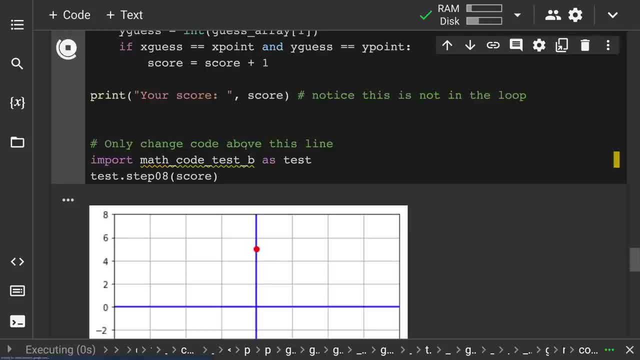 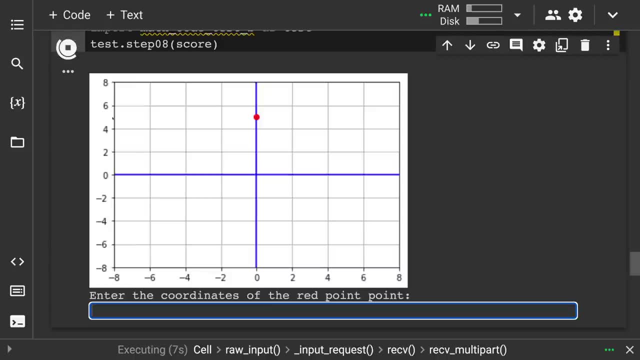 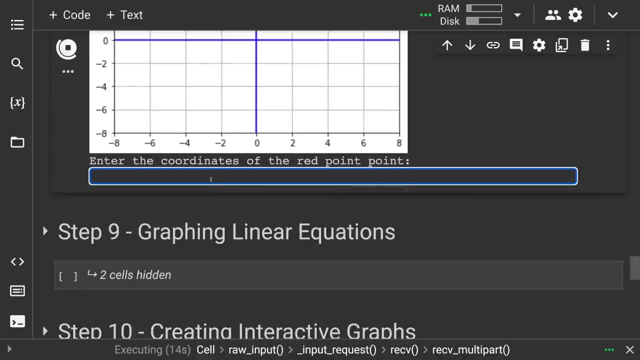 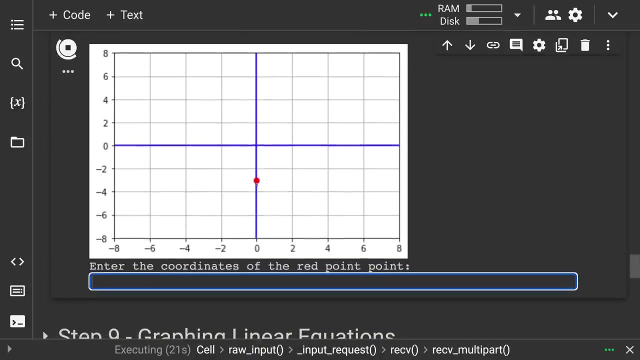 Initialize it at zero And we'll see, see what happens here. So you see, with the grid lines we can see: So zero, and Look at these: four, five. So the coordinates of the red point would be zero, five, And Here we have zero. 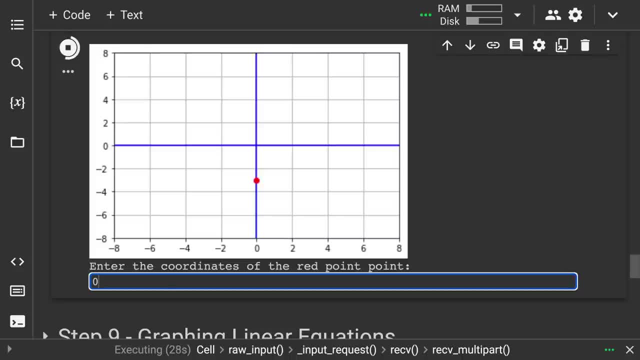 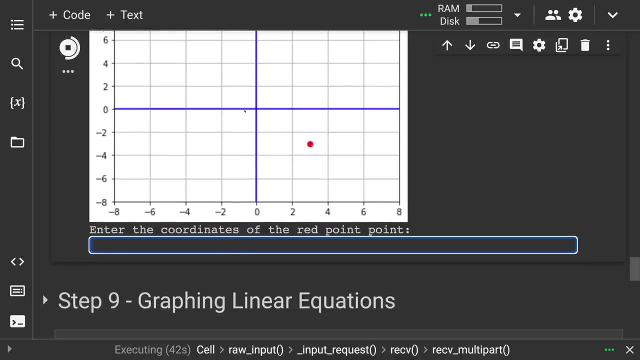 Negative three: Zero Negative three, And this is why I made it eight in every direction, because it actually the grid lines just work out a little bit better. So what's the coordinate of this point? so looks like three on the x-axis and then down three, so that would be three. 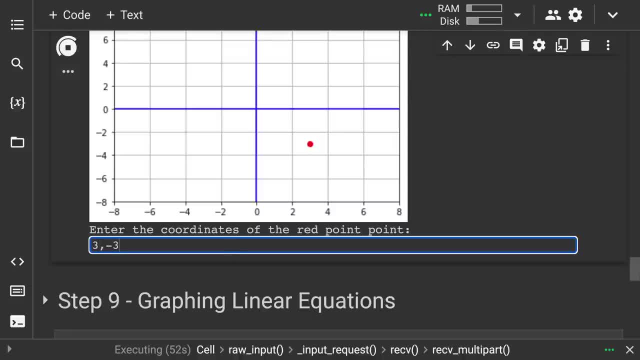 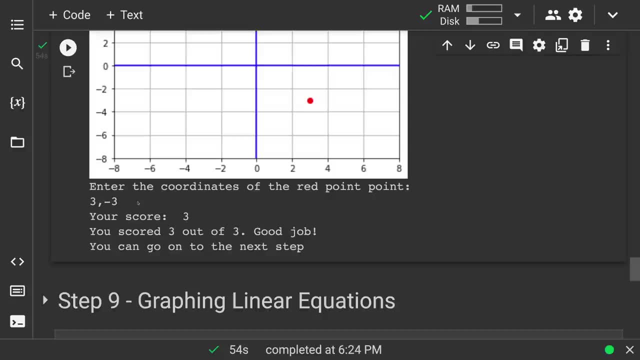 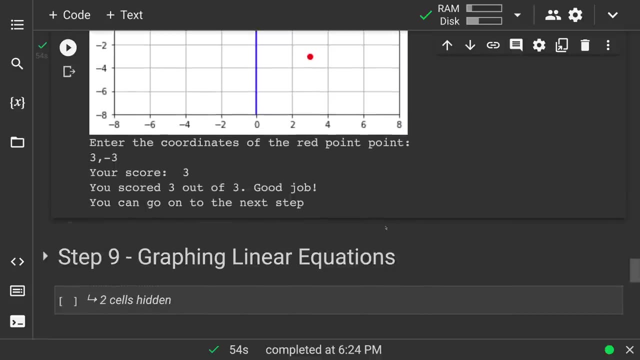 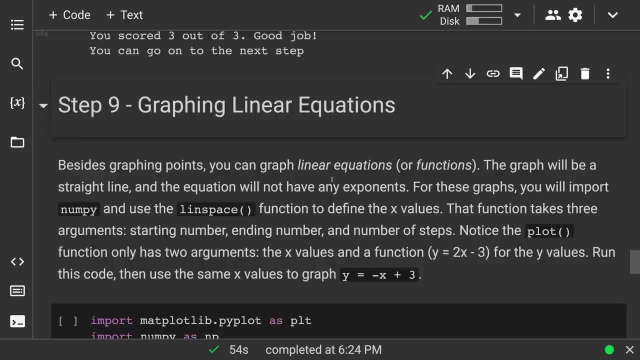 Negative three. All right, and There we go Can try this out. It'd be a good way to Test your understanding of coordinates. All right, and step nine. so now if I want to graph a whole linear equation. So this was nice if I define these two points. 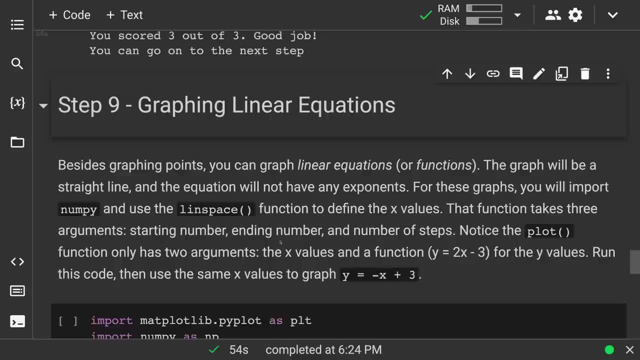 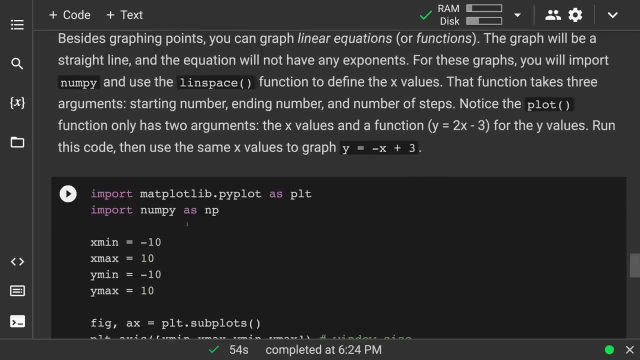 And I can draw a line between them. but what if I actually just want the whole linear equation? So NumPy is the library we're going to use for that. So we're going to import NumPy as NP. now that one. I mean NumPy, not that big of a word to write, but 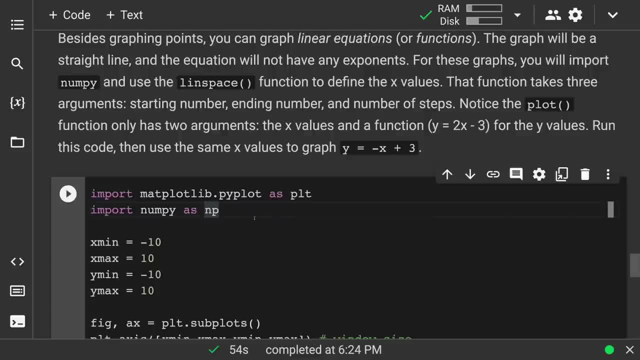 As NP. it just seems to be a common thing. so you will see NP dot this or NP dot that for the different functions, All right. and then we have the Lin space Function. so that defines an array of values. When we're talking about functions, we can, you know, loop through, but this gives us that array. 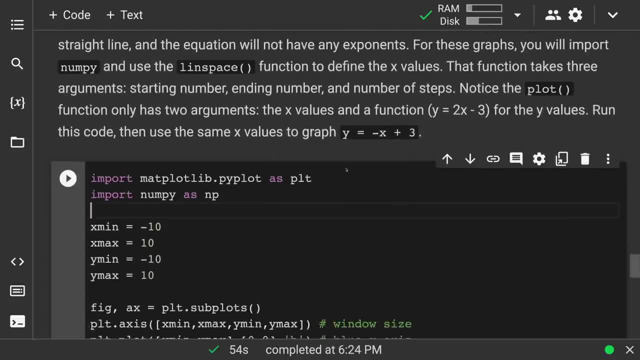 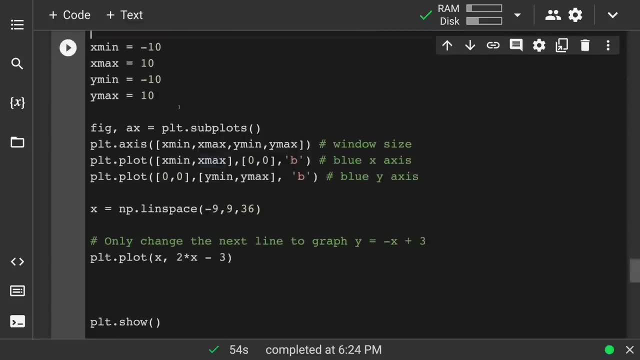 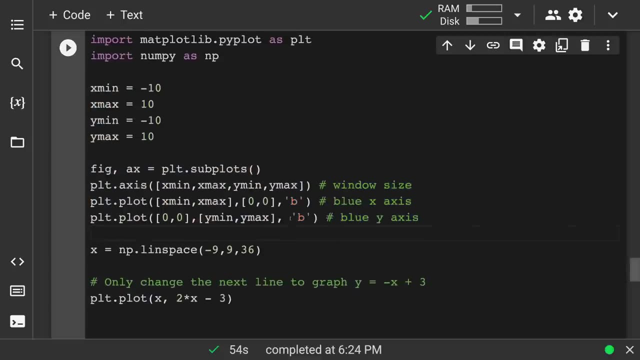 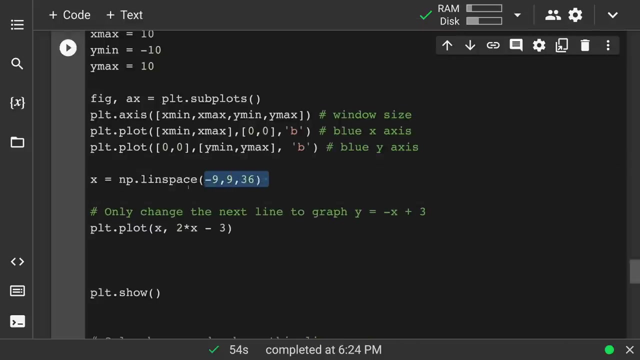 And we're going to plot the function With two arguments. So If we take a look at this, all these, so after we important on by Same setup for the graph And then Lin space, We give this. Now I purposefully made it a little bit less- you actually will get to some other things that we can do. 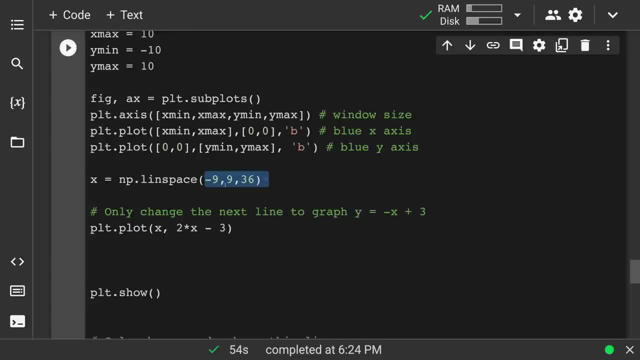 What with this? that will make it even better, but I made it Purposefully a little bit less than So. Maximum values here on the graph and then the third argument: so it goes from It's the X values is what we want for this. so the X value goes from negative nine to nine, and in that there are thirty six points. 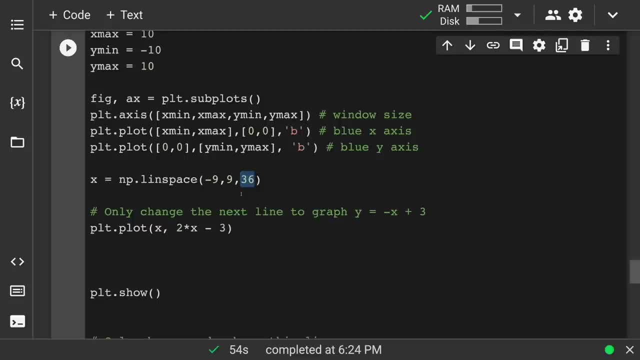 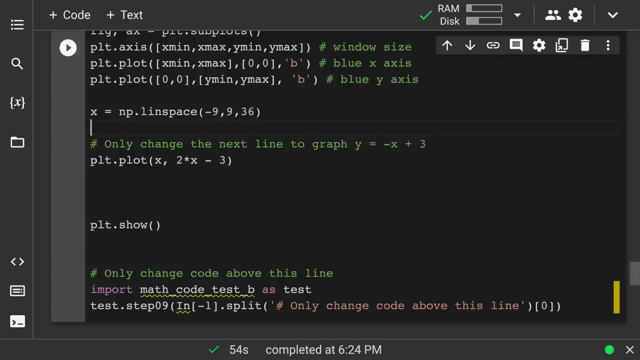 So, Believe it or not, that's actually going to be enough, which is: you know four points. You know like every one fourth is a point. That's actually going to be enough. And notice then what we're plotting here: Our X values. 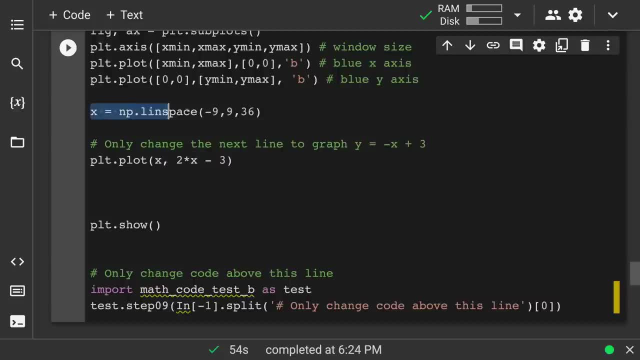 And you see, that's the array of X values. NumPy gives us that array, So that X values, and then, Given this, I can just put this equation in here As that's the Y value each time, So, as it goes through this array of X values, that Y value. 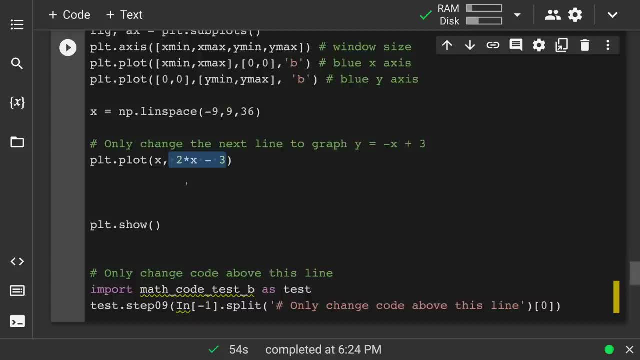 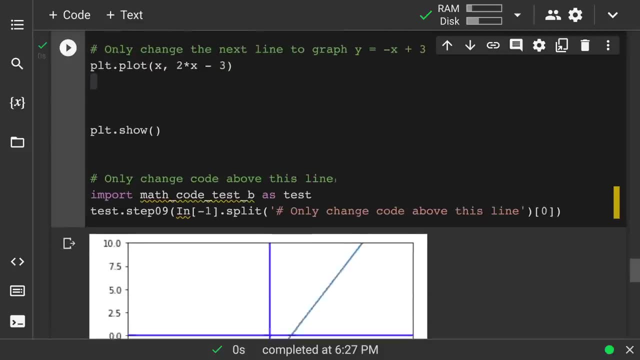 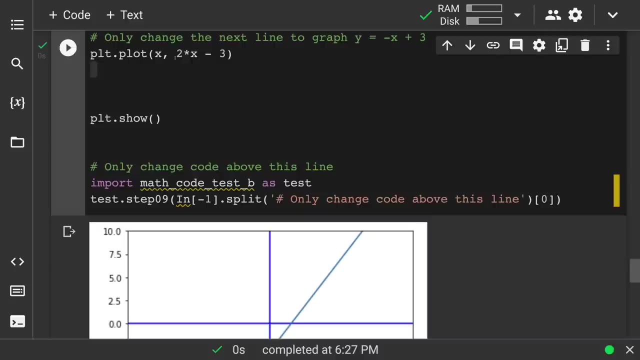 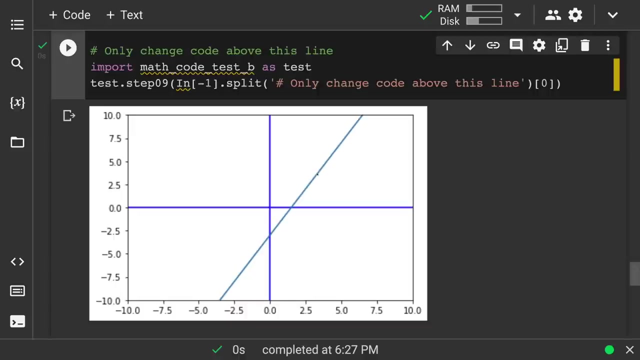 Is going to And It calculated each time and then that's what it's going to plot. So Then when we run this, We see that it actually plotted this point, this, this graph. There we go Two X minus three And it looks like it crossed there about negative three and looks like about up to everyone, cetera. 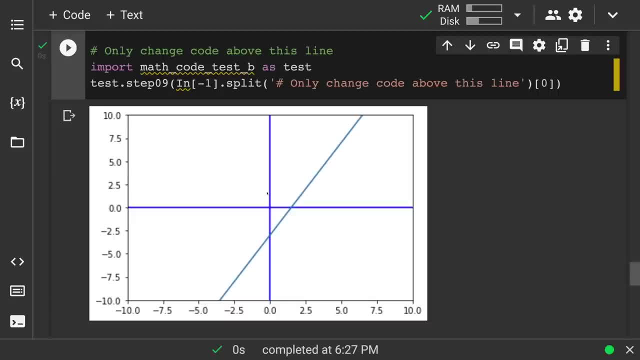 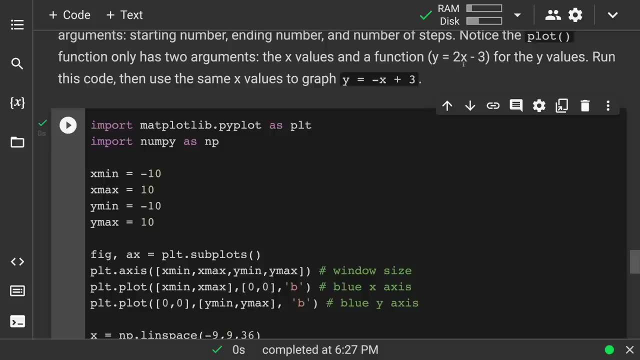 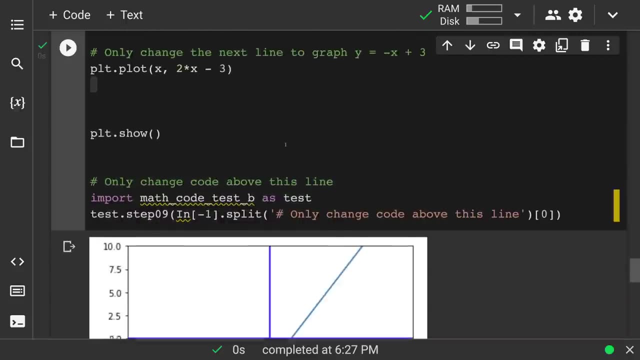 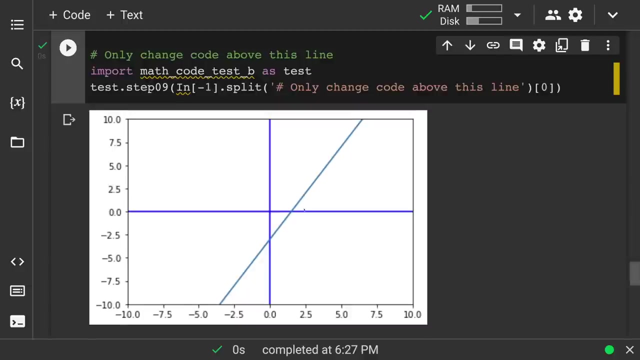 Okay, So There we go, And We have this run it and then change it to graph negative X plus three, So all these can stay the same. Now, in this case, Since this was cut off here, we didn't really notice that. 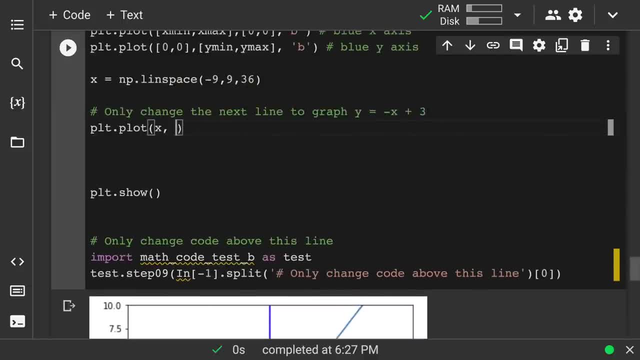 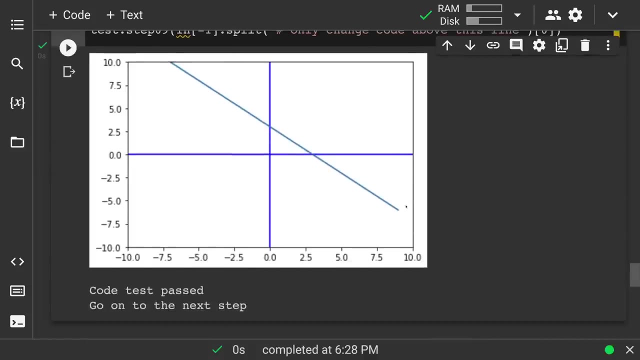 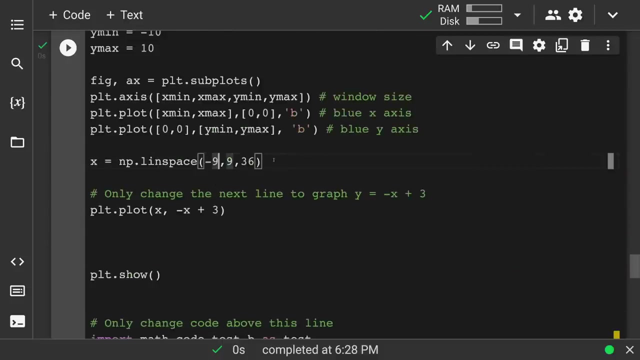 But if we just then change this To negative X Plus three, Now we see The The limitations of this, Because It cut off there. So what can we do here? Well, We could, We could In this. 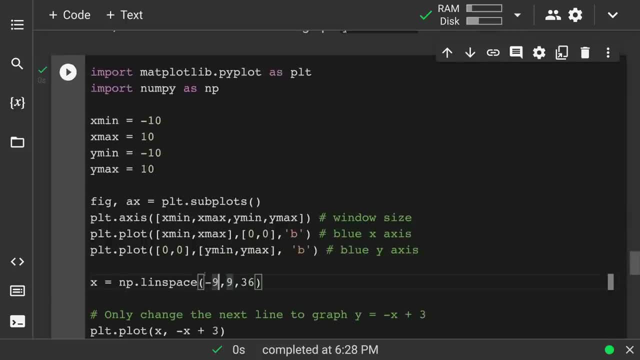 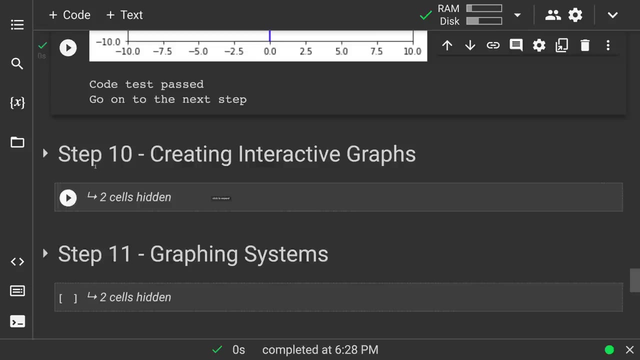 Just Make this. we've already defined X min and X max. we could actually make this Go from X min To X max And you'll see this come up in the next things we do. All right, So We can create interactive graphs. 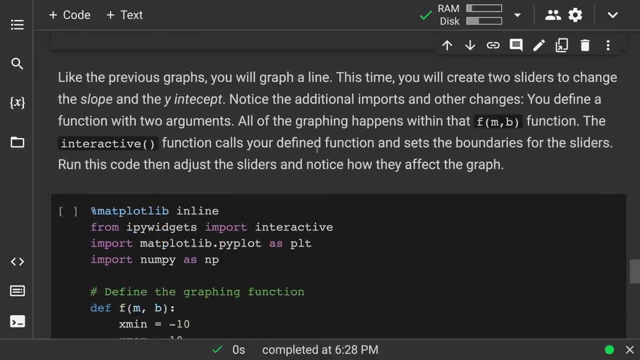 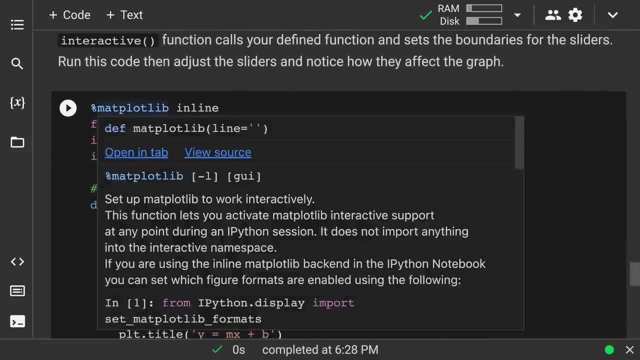 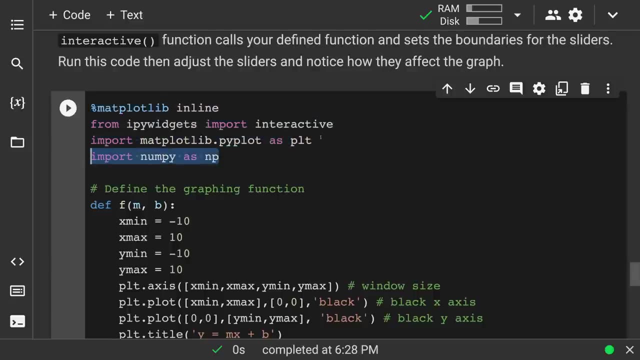 So In this case We've been talking about linear equations. Let's, let's use these widgets to make a slider, So we're going to import all these things here Now. You know, numpy for our array of X values, That plot library for the 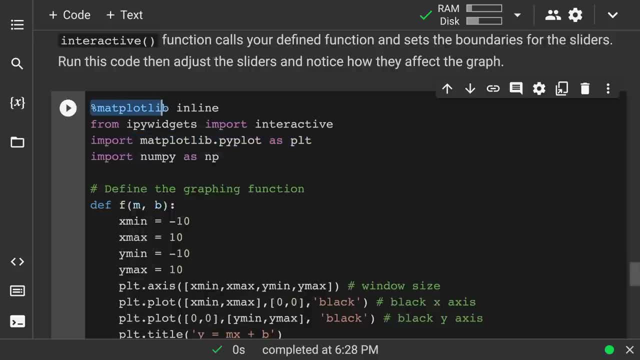 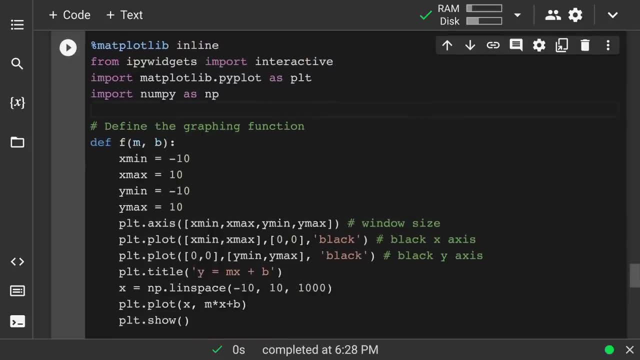 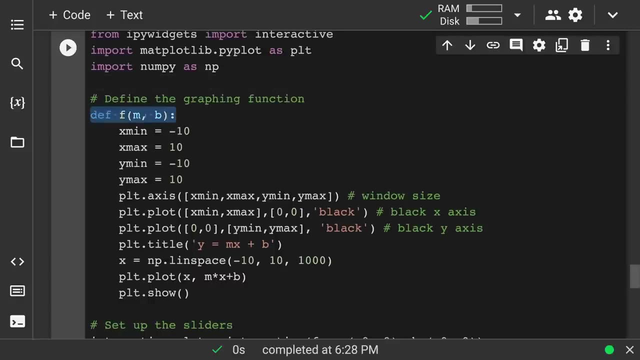 The plot, And then we have- We're going to import this in line- and then the widgets, So We can make All the graphing happen in a function. And we have. There we go, Function Then be, And 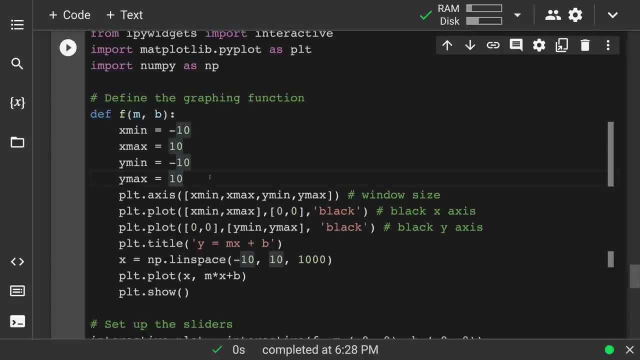 If You, If you, were working through some of the other things In this course, This might be Familiar and then we'll see. just You know What's The same and what's different about what we're doing here with this function. 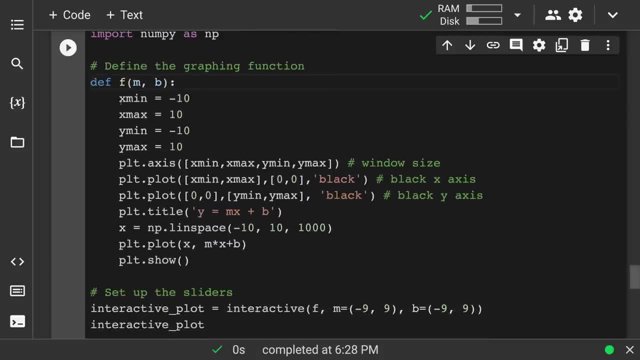 So, If I have this function of M and B, Everything Happens in the function Defining the X values. Why Maximum Defining all of this? And In this case We're going to give it a title because 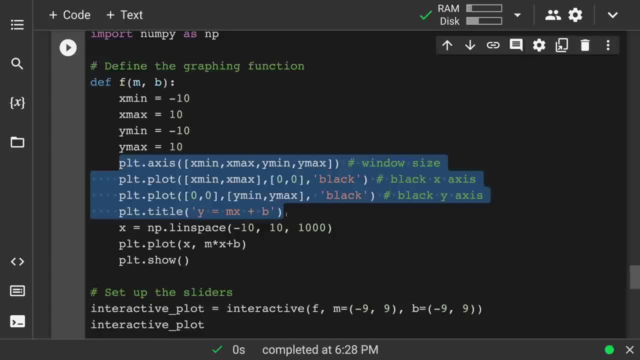 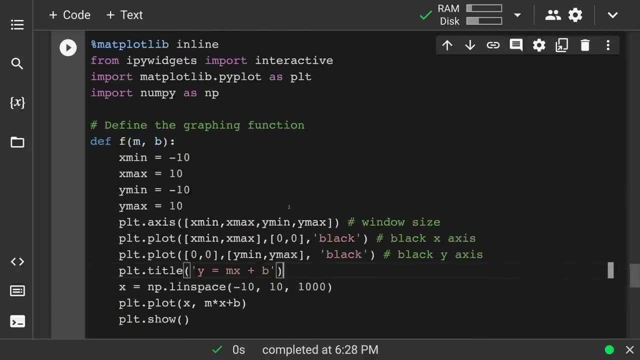 We already know that this is going to be a slope intercept equation, So we're going to give it that title, All right. And then we have, There you go, NP dot Lin space, And We could Always Make this now. 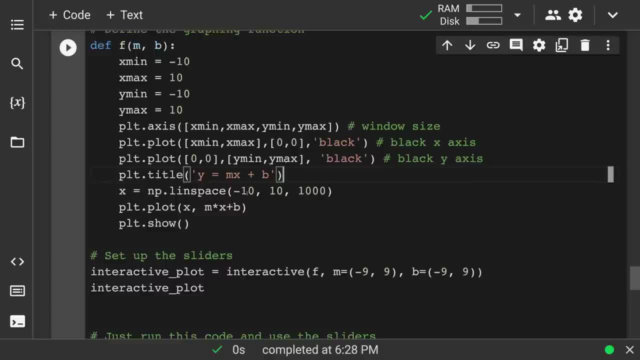 This time I also rewrote the numbers, but you could always make this Just X min, X max And Something else here. So What are we going to do here? We're going to plot X And then. 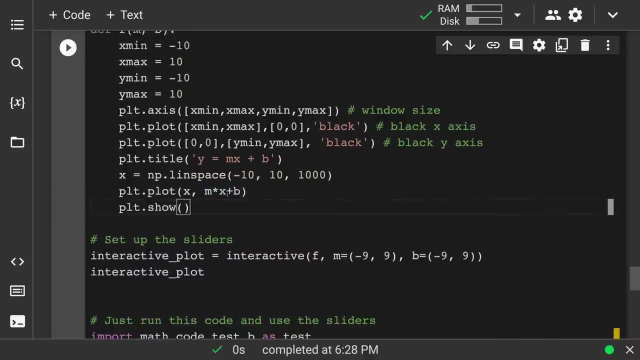 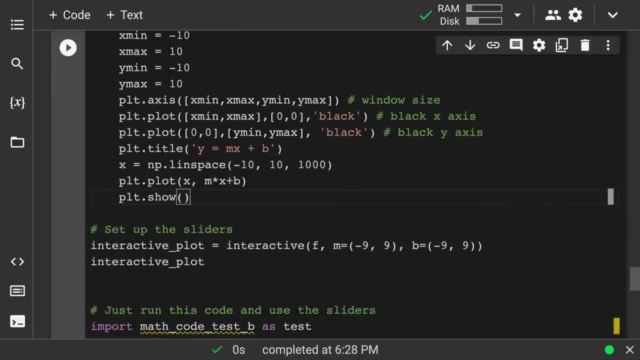 MX plus B, Because These M and B values are going to come from Slider And then The function is going to Take that. So Here's our interactive plot. I mean I could have made the variable something different. 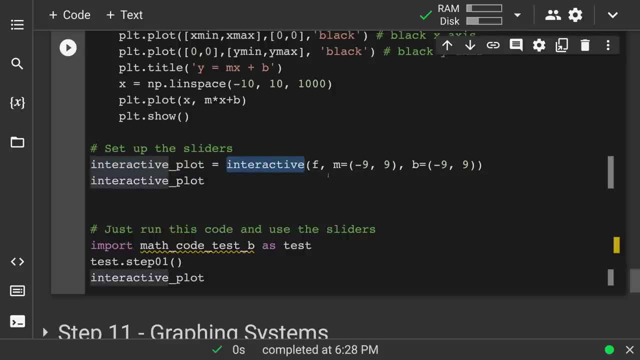 But The Function is interactive. And then It takes F- What's What function? And then M equals. So we give it a range And B equals, And we give it a range And we run this interactive plot. 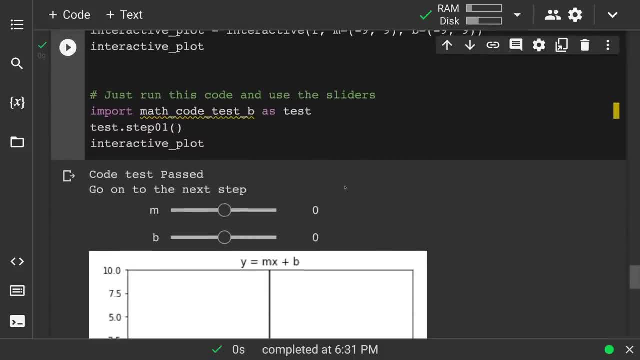 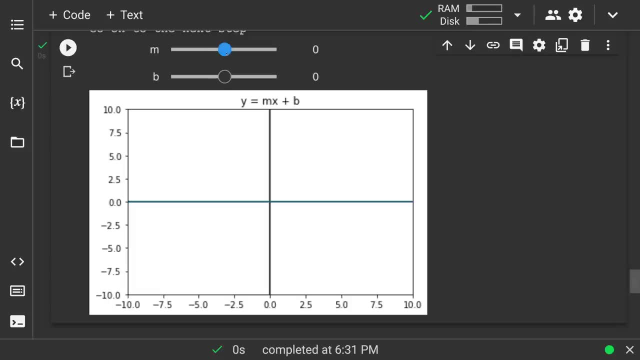 So We can use this. The plot Now- notice It- Default goes to zero. So As soon as I increase M, You see Now I have a line with a slope of two, Line with a slope of four, And then 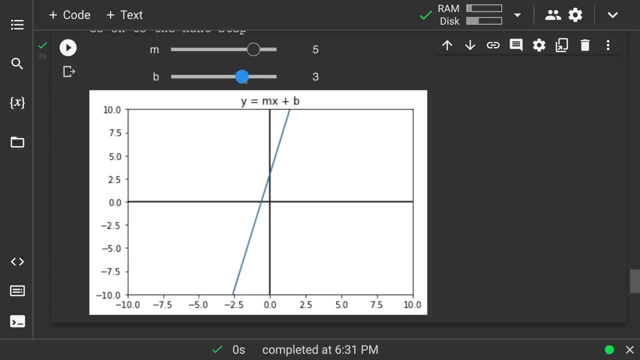 B is still zero, But I can move this up And I can move it down And we see That I can adjust my graph. So It's nice to have these things, that we can adjust A graph- All right. 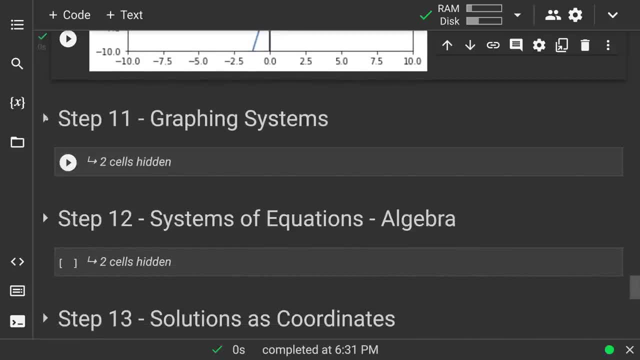 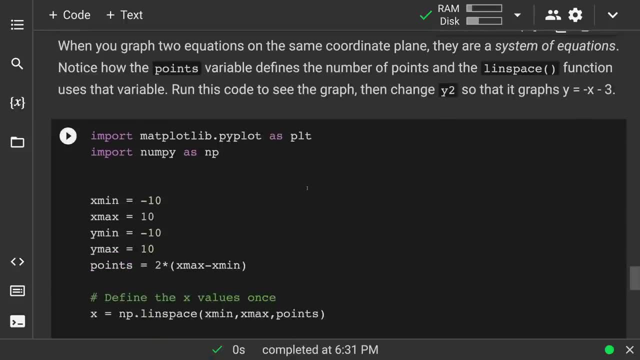 And then If I'm graphing a system, So Maybe You are already graphing System of equations- That Then Hopefully This is A good review. If this is new, Then Take a look at. Here's one way to graph a system of equations. 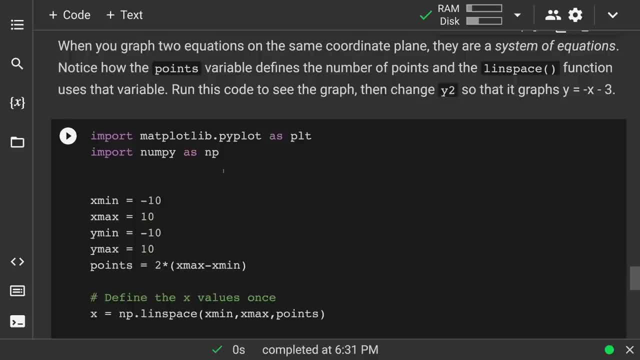 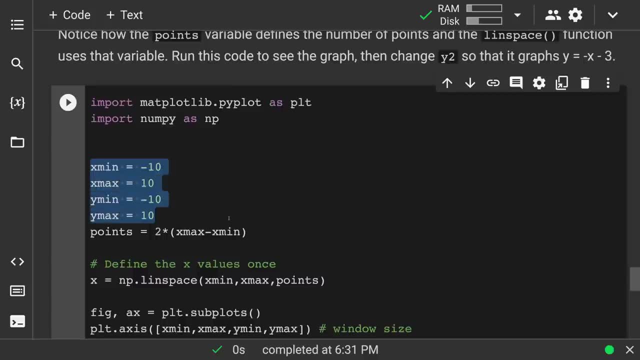 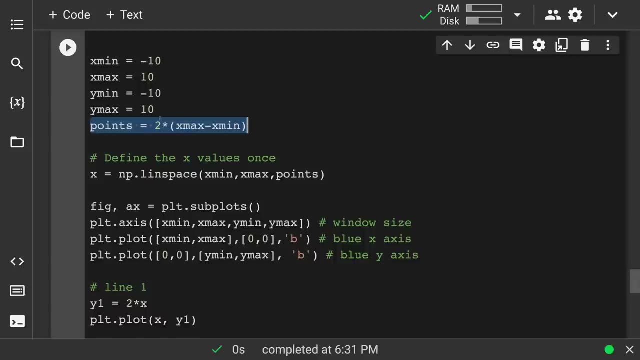 All right, Same imports And Same defining These. Now Here's where We make it A line, And It Goes A lot Better. So How Many Points Do I want? I'm 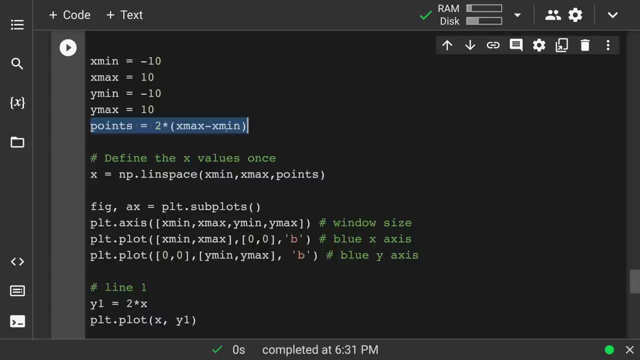 Just Going To Take It Also Based On This: X Max Minus X Min, So That's Going To Give Me. So That's How Many. 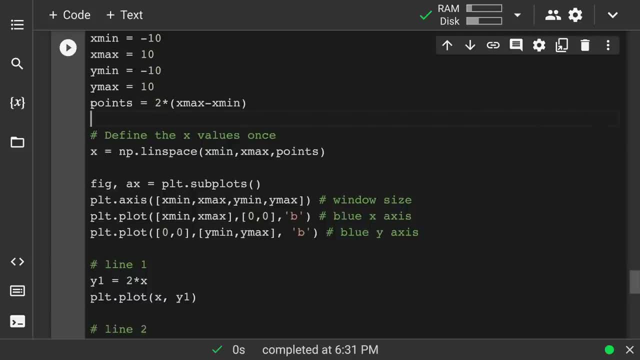 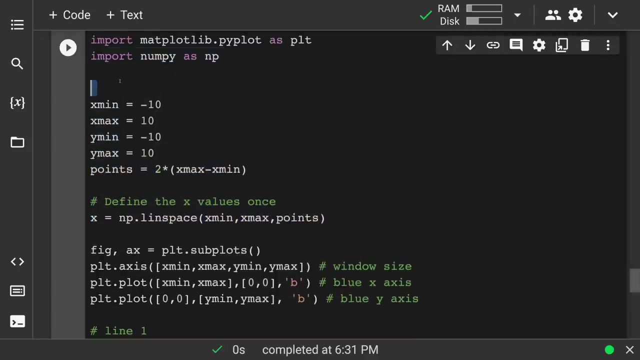 Points. I Have That. You Know, There's The Range And Then Times Two And Then Define The X Values Once, And Here We Are Defining. 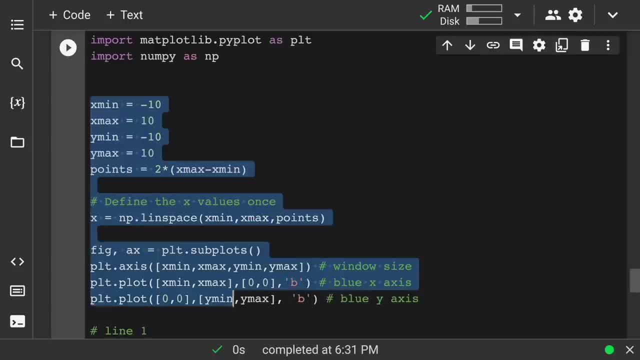 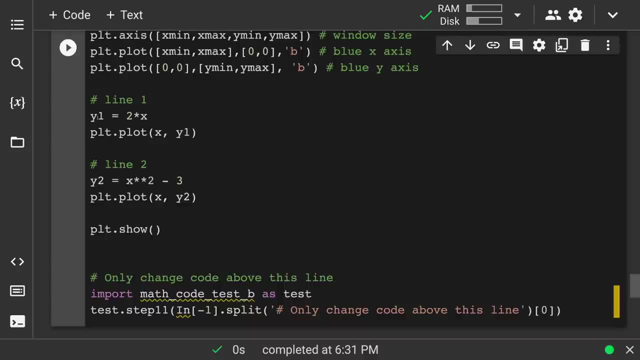 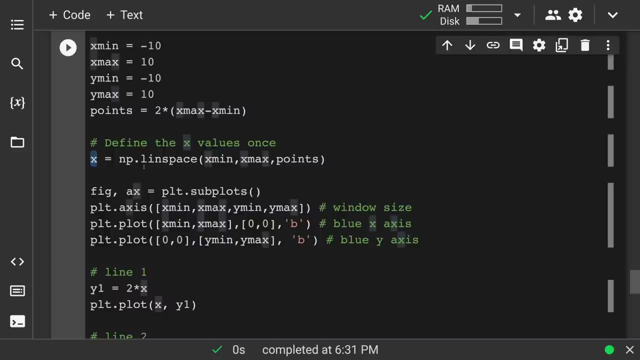 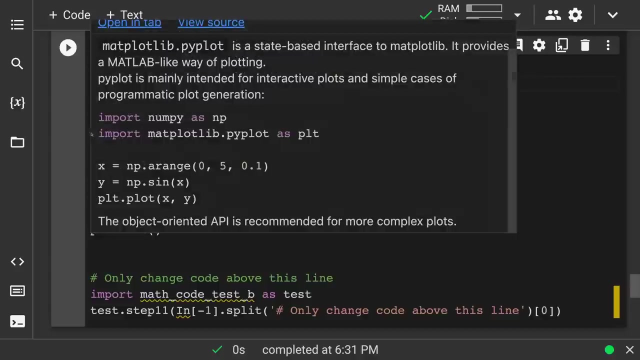 Our Base Of What We're Importing And Then The Basics For The Graph. So Then I Can Plot Two Lines, You Know, Define Why One. 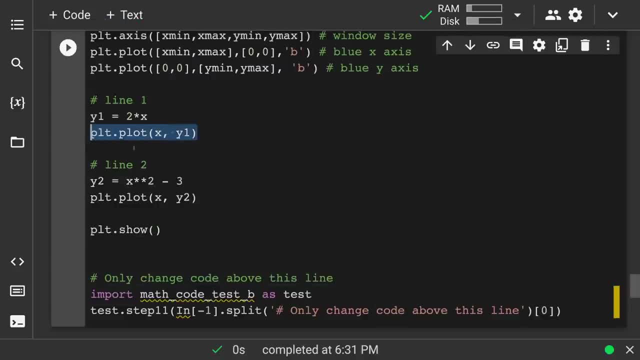 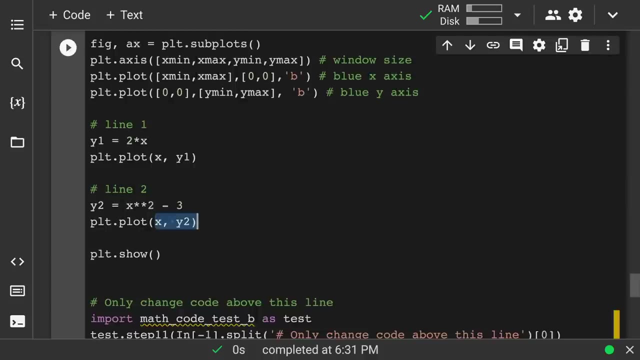 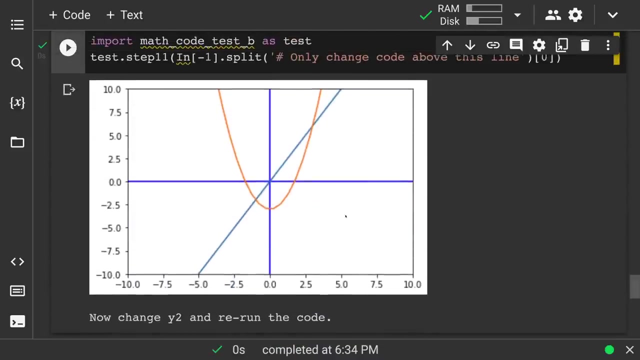 In Terms Of X And Then Y, One. There We Go, And In Line Two. Notice, It Doesn't Have To Be Linear. This, This Plot. 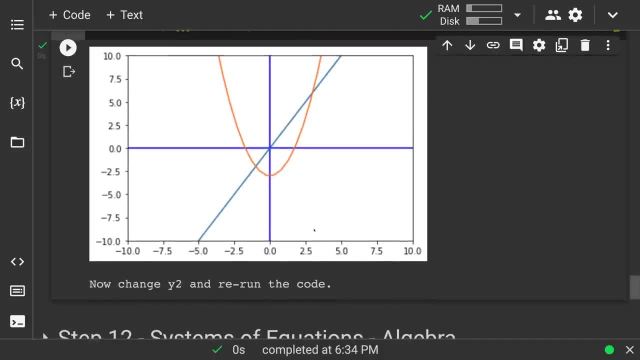 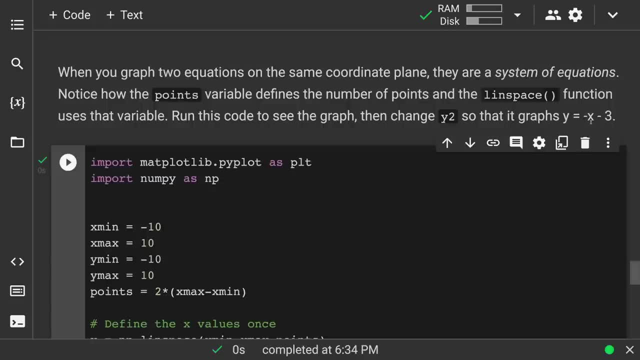 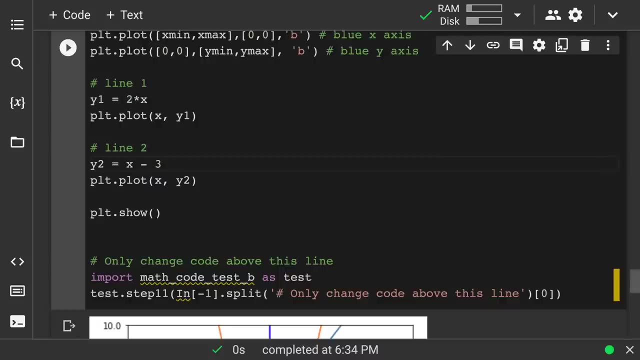 Works. You Know, X Square Minus Three. And So Why Two? We're Going To Make It Negative X Minus Three, So We're Just Going. 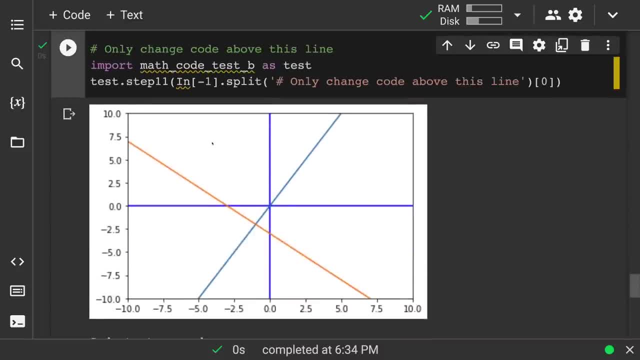 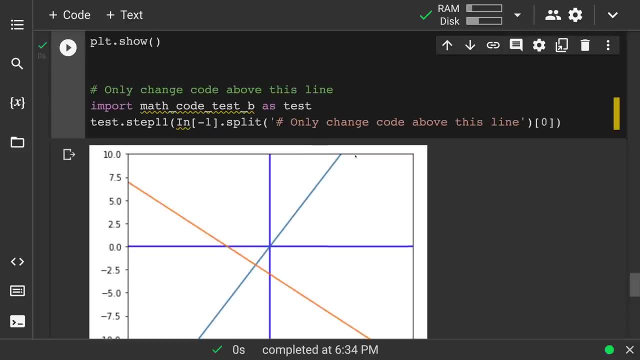 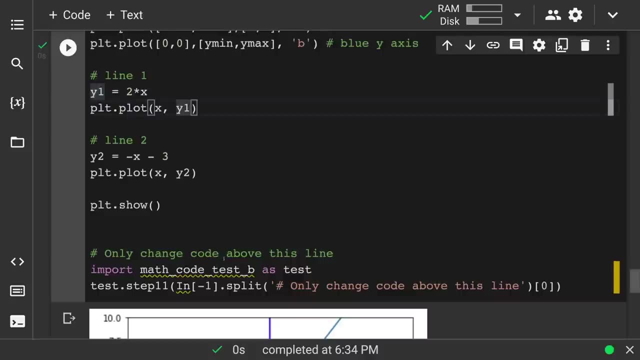 To Rerun This As Negative X Minus Three, And We See, There We Go, Linear, Linear. It'll Go Through A Few Colors And There 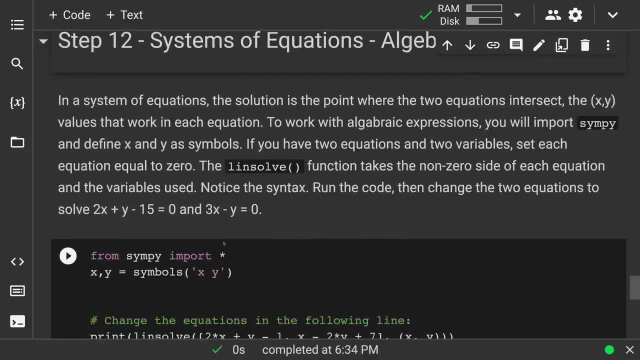 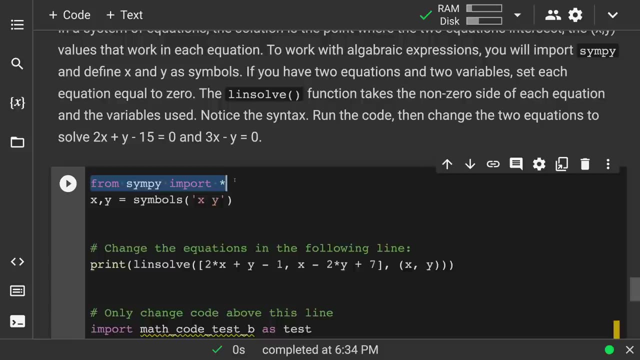 We Go Defining Two Points. So Systems Of Equations, You Know. So There We Go. That Was Graphing Two Equations Probably Don't Need. 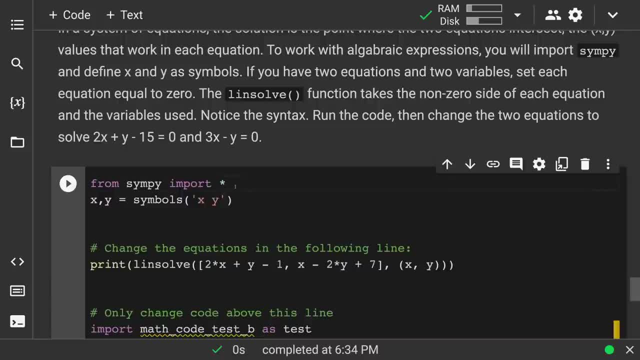 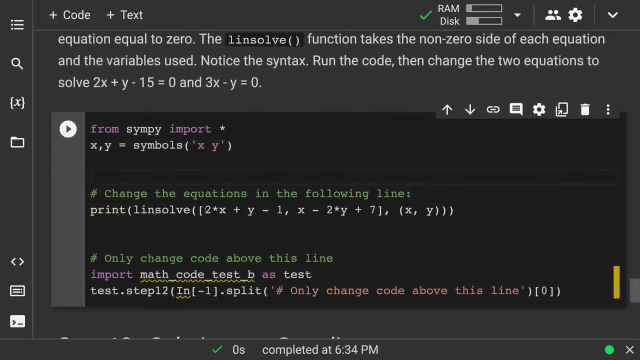 Import Everything, But I Do For This Particular Example. So The Import Asterisk Is Going To Import Everything From The Sympy Library And We're 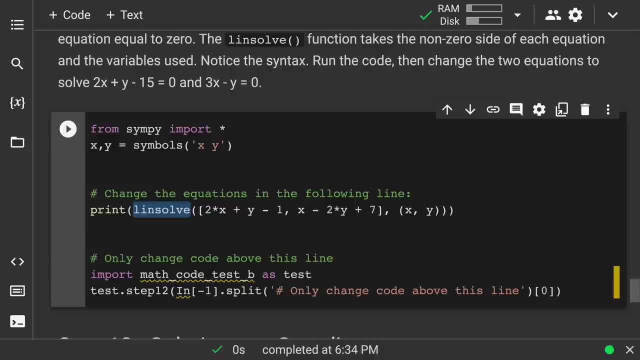 Going To Solve Notice Open Parentheses, Because That's The Function For Lin Solve. And Then What Do I Have? I Have This Array Of These. 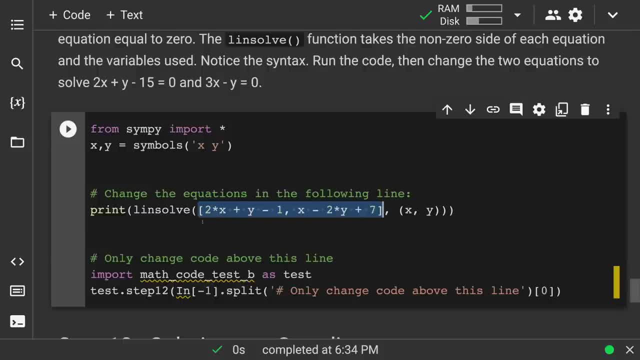 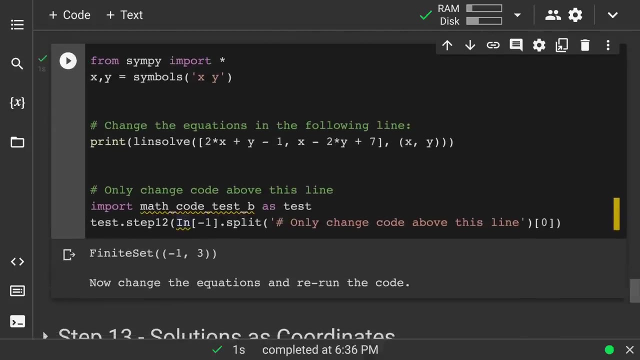 Two Equations Set Equal To Zero. It Would Be Those Set Equal To Zero. And Then I'm Solving For The Variables X And Y. 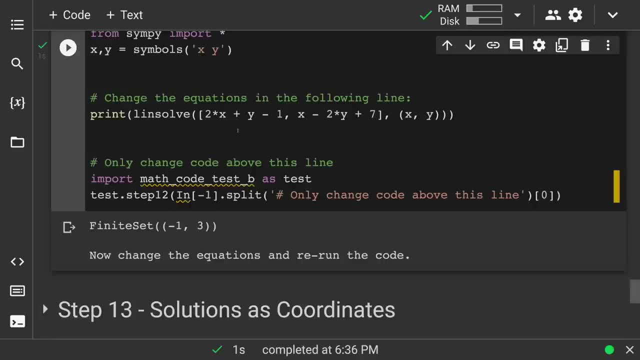 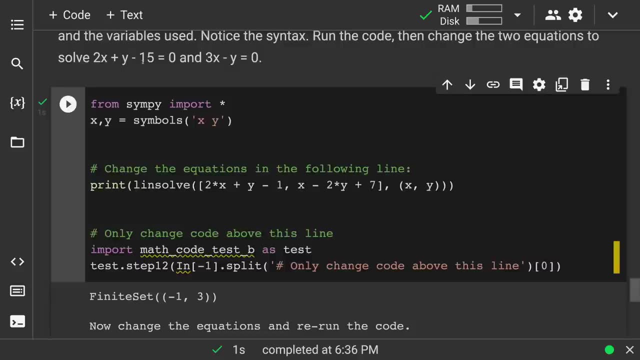 And What Happens When I Run It? It Gives Me This X Plus Y Minus Fifteen Equals Zero, So Two X Plus Y Minus. 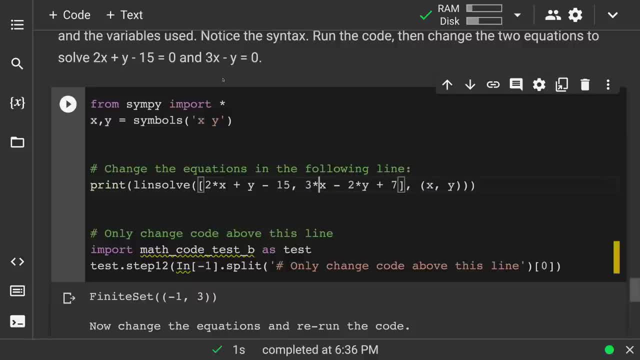 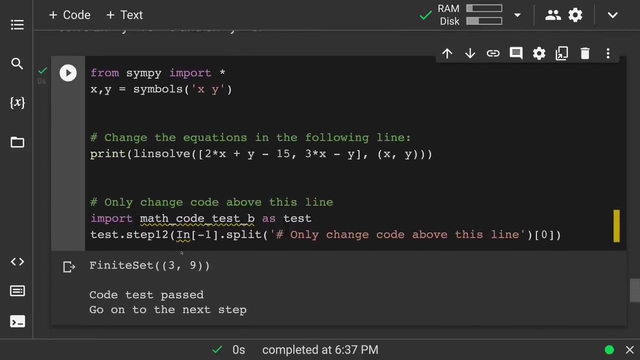 Fifteen, We'll Just Change That- And Then Three X, So Remember Three Times X. You Know Zero. So There We Go. And If We Run, 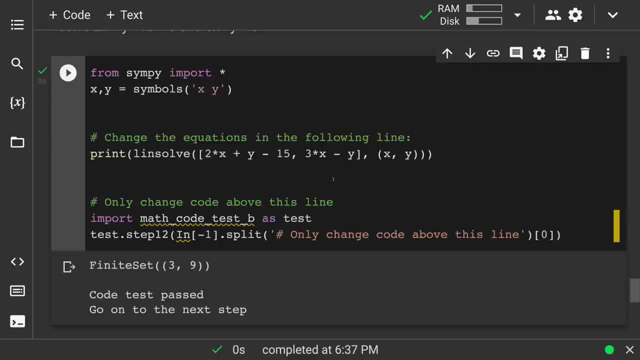 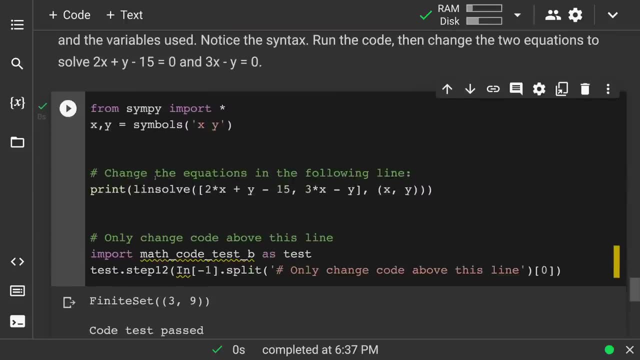 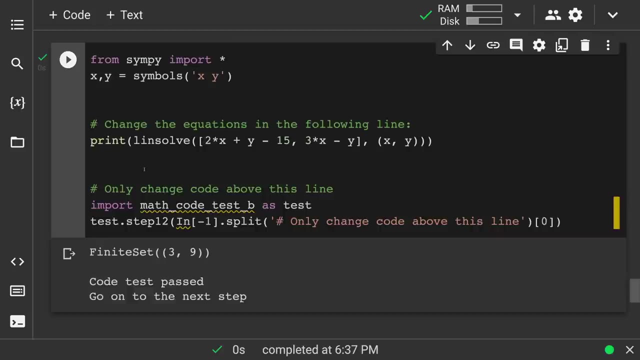 That There We Go. Three, Nine Is The Solution. So There You One Way. One Of The Way Is To And Output. You Make The Output. 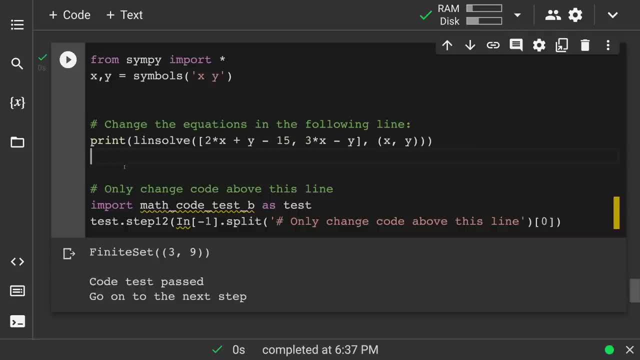 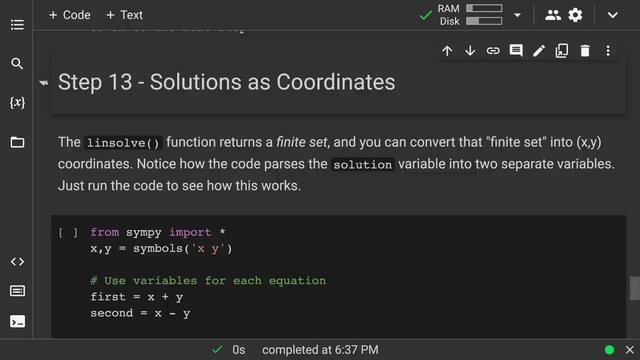 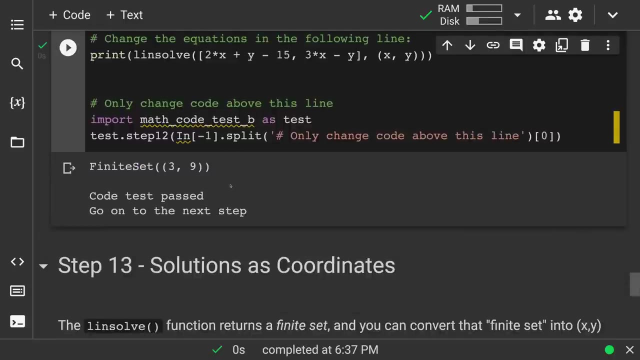 Even You Know A Little Bit Nicer. So If You Haven't Already Gotten To That, You Will. So Now We Can Get The Solution. 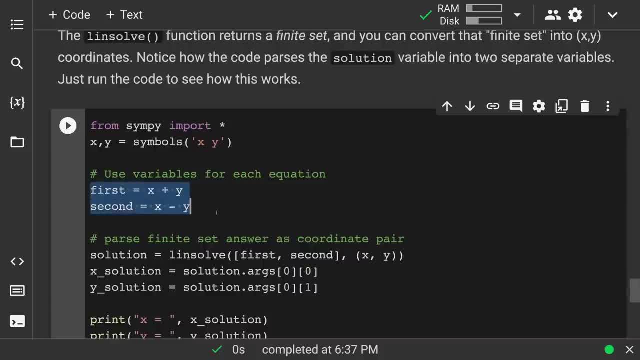 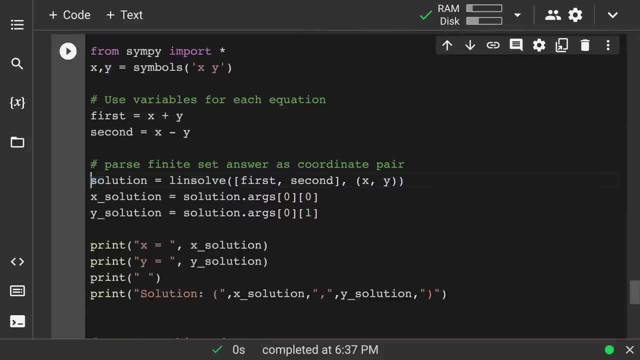 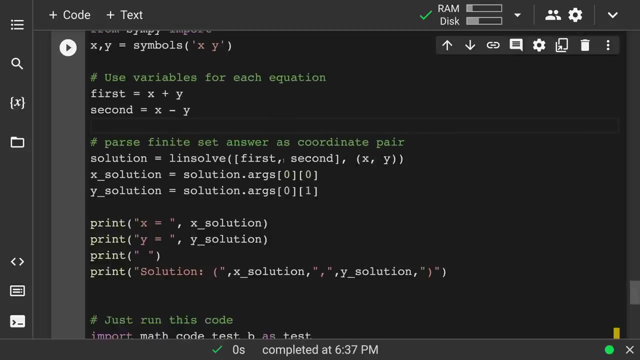 So Also Here I Split Out First And Second As Two Different As A Way To Put These Here. So Now, When I Have This Solution, 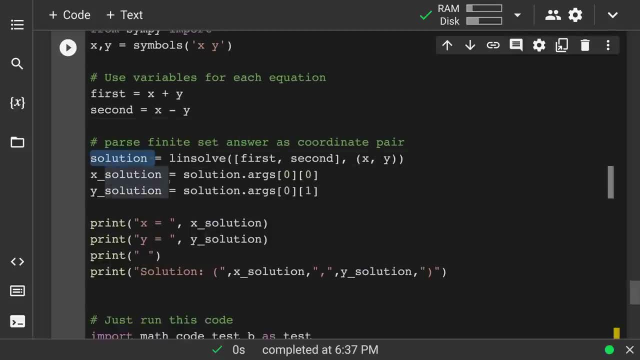 I Don't Have, So This Is How We Parse It Out. I'll Call This Variable X. Solution Is Solution Args Zero, Zero, And Then The 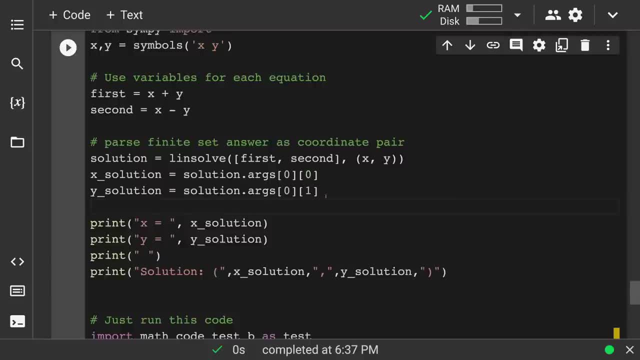 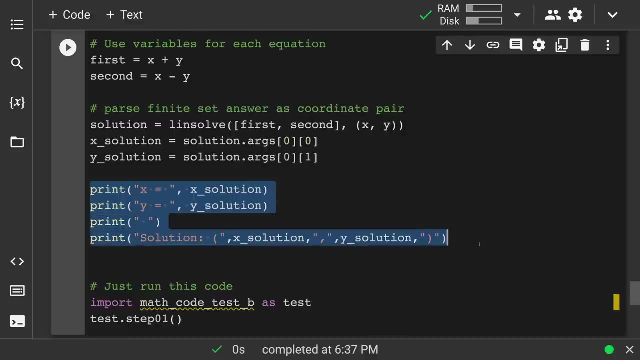 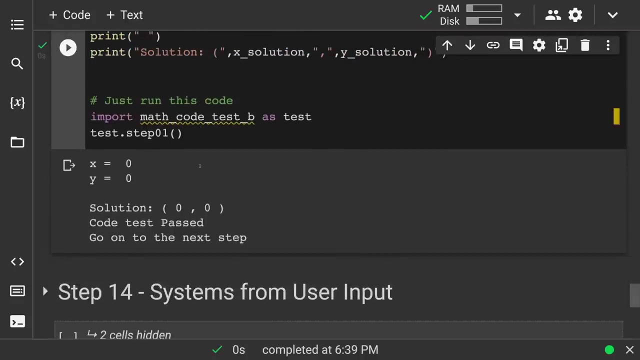 Y Value Is Going To Be Solution. So Now I Have These As X Solution, Y Solution And I'm Going To Print Them Out. X. 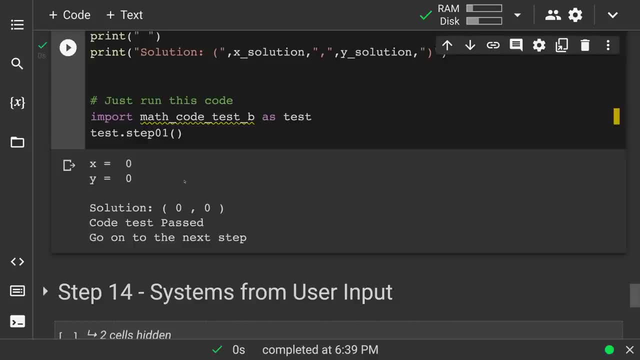 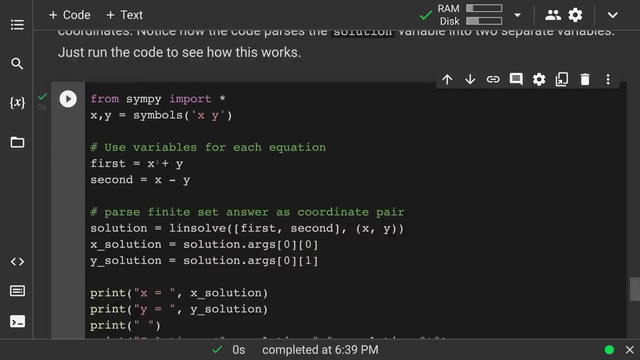 Equals, Y Equals. And Just For Kicks I'll Also Print It: X Plus Y, X Minus Y, So They Would Cross Zero, Zero. So 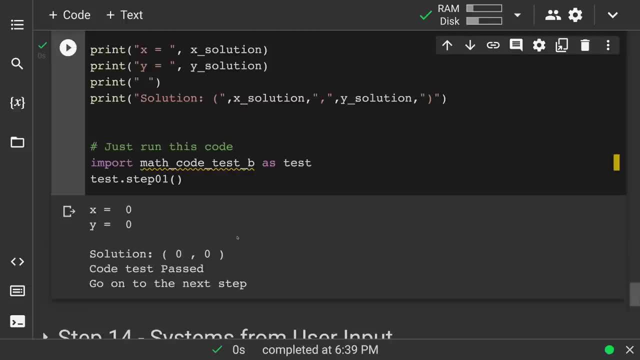 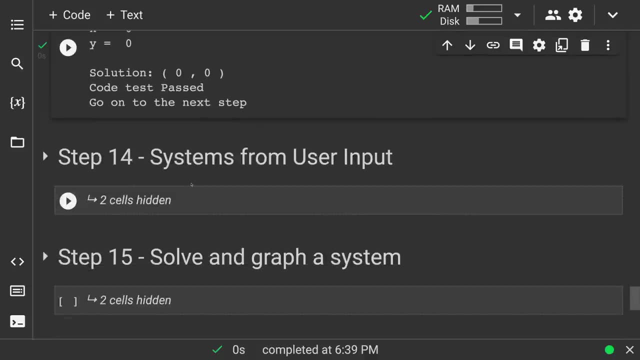 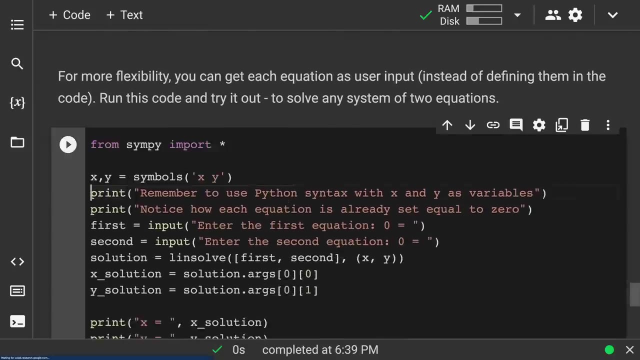 There You Go Again, Another Way To Then Elevate That And Solve It. Just Showing You Different, I'm Going To Print For Anybody You. 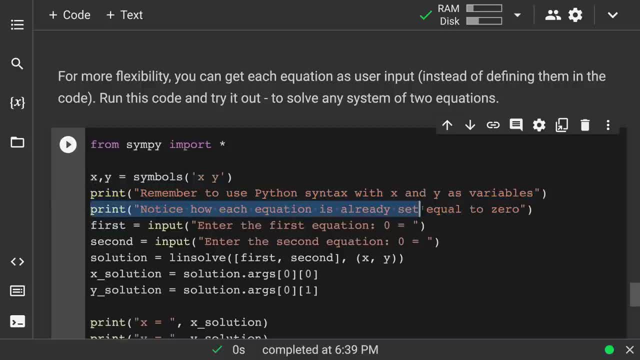 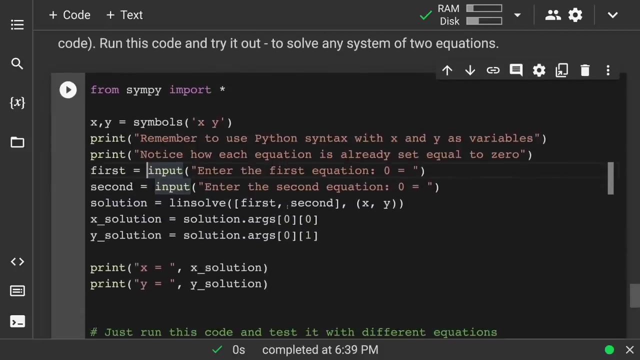 Know This, Remember, Use Python Syntax And Then Notice How Each Equation Is Already Set Equal To Zero. Because I'm Going To, Then Lin Solve. 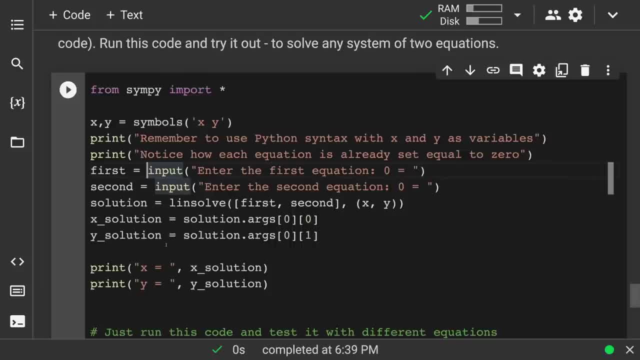 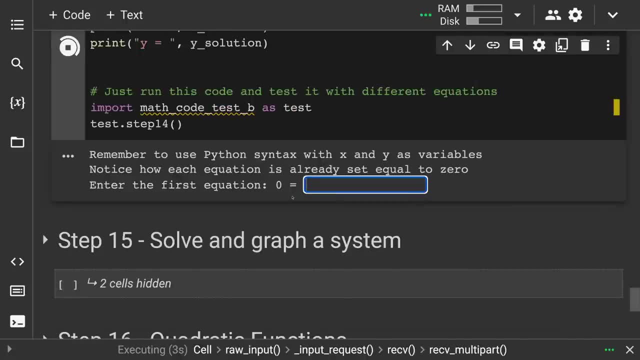 Works Out Like That: There You Go First, Second And Then Parse The Solutions, So Let's Do This, As Long As Long It's Two Things. 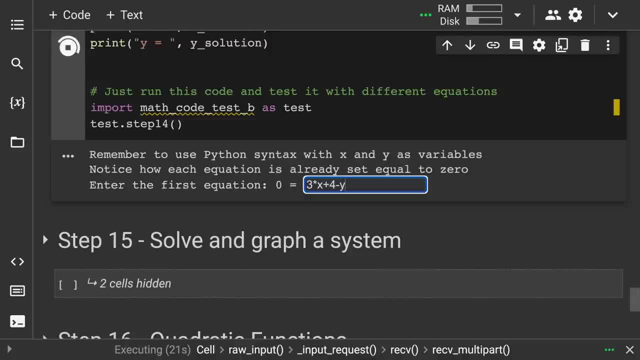 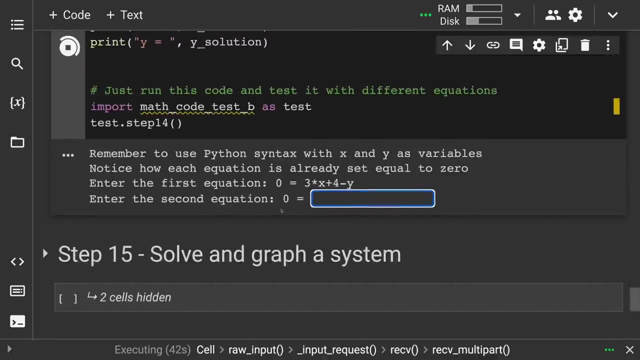 Set Minus Y. So If You Think About Things In Terms Of Y Equals, Then You Could Just Put A Minus Y Here, So Three. 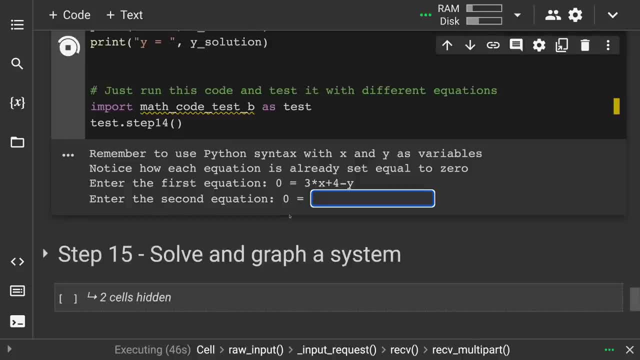 X Plus Four Minus Y. All Right, So What If I Have Five Times X Um Plus Five? We Go And Notice The Space Minus. 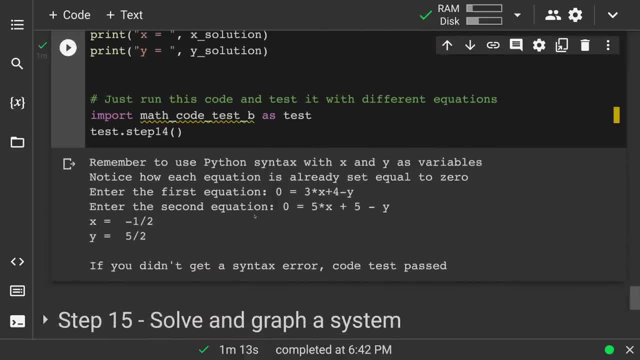 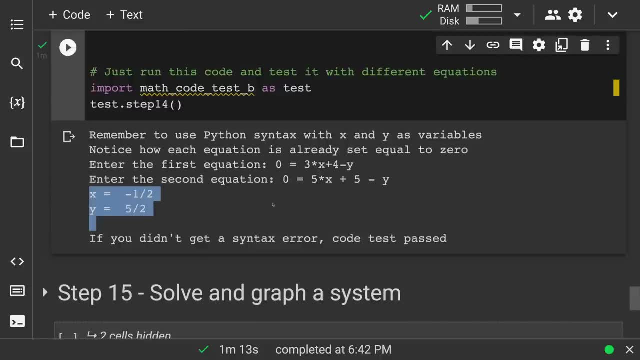 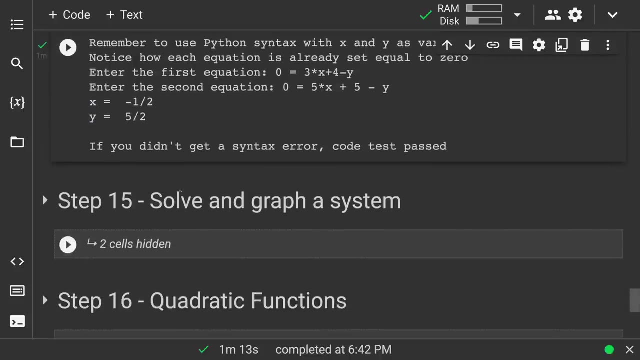 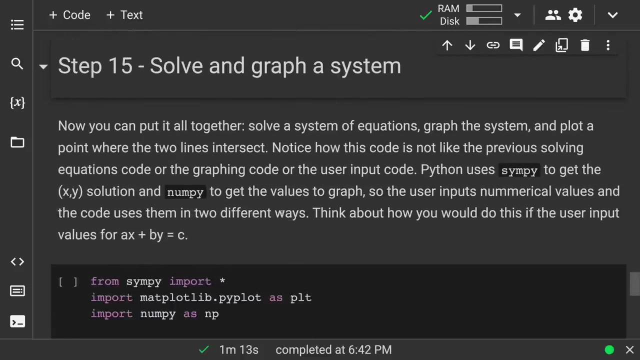 Y We Go. Hit Enter, There We Go. We Have An X And Y Solution. Pretty Cool, All Right. And Then Solve And Graph, Which, In 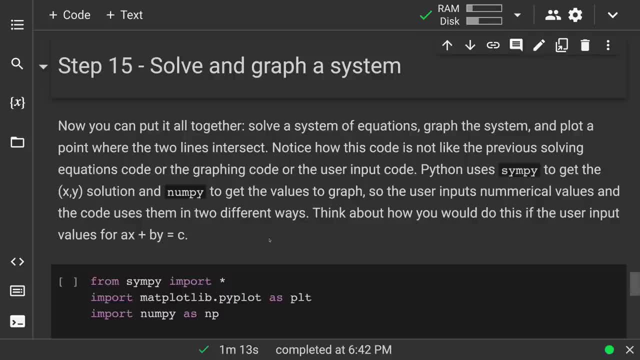 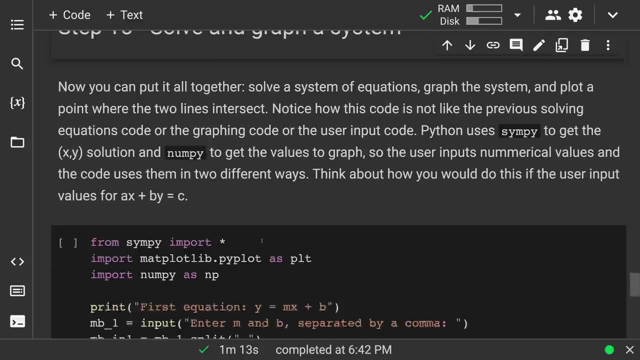 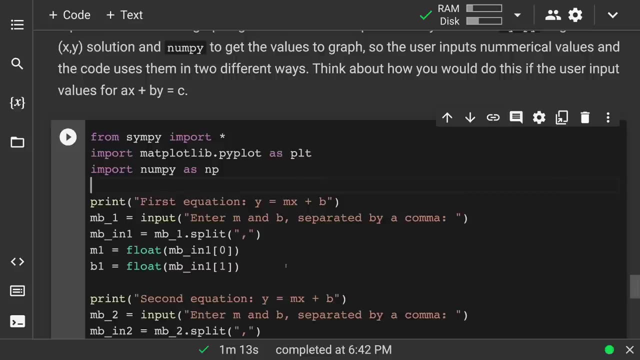 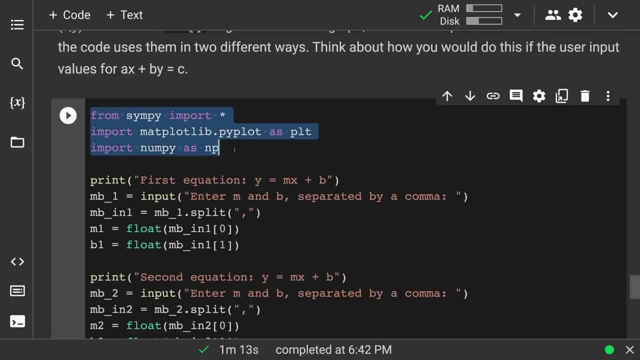 In This Whole Course, The Solve And Graph You Know, You Get More And More Familiar With All The Different Ways To Solve And Graph. 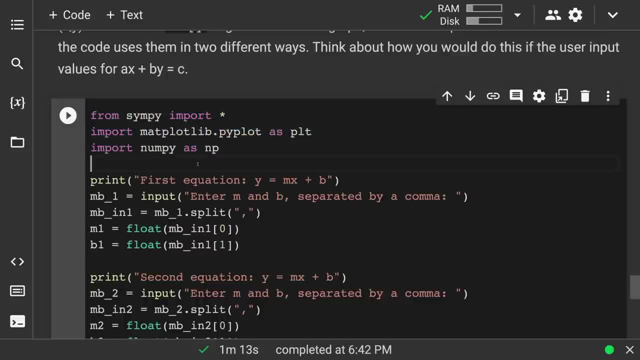 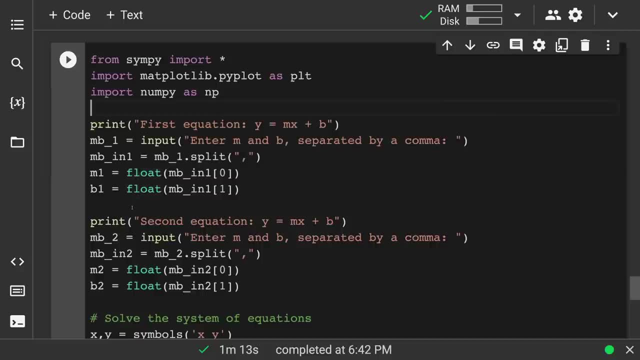 Then You'll See That We Can Get More And More Elegant Solutions With Linear Equations And Knowing That It's Linear Equations, Notice I'm. 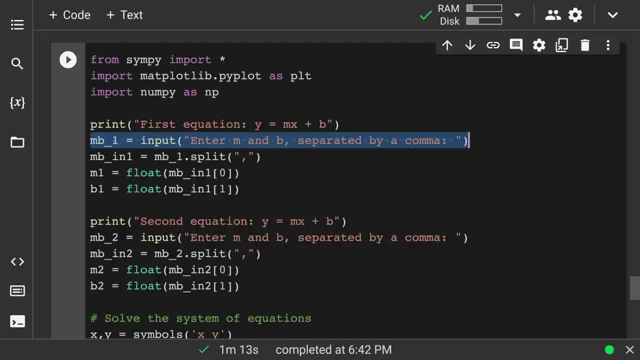 Only Asking For M And B Separated By A Comma, So I'll Call That Input M B One, Because I Take The First One. 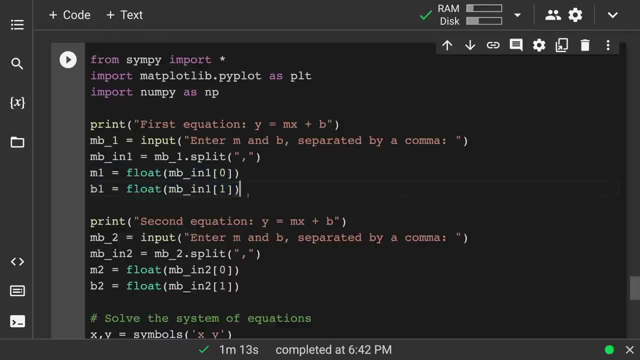 And That Must Be M, And Then The Next One That Must Be B. So We See That. You Know, Take This Input, I Will I. 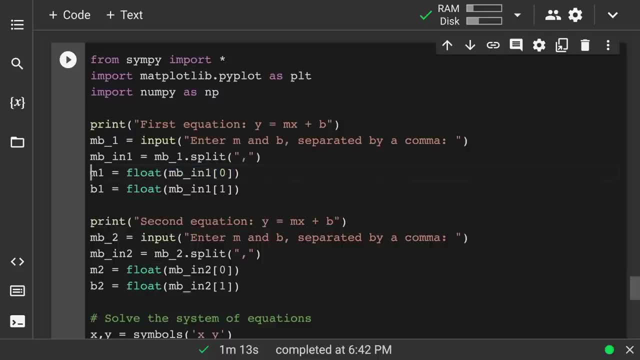 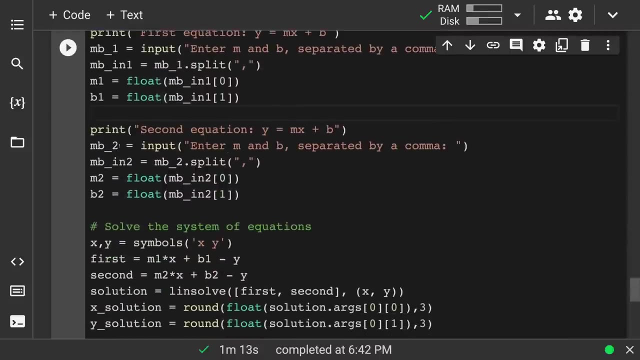 Have A Element Zero I'm Going To Cast As A Float Called M One, And Then Element One, The Second Element I'm Going To Cast. 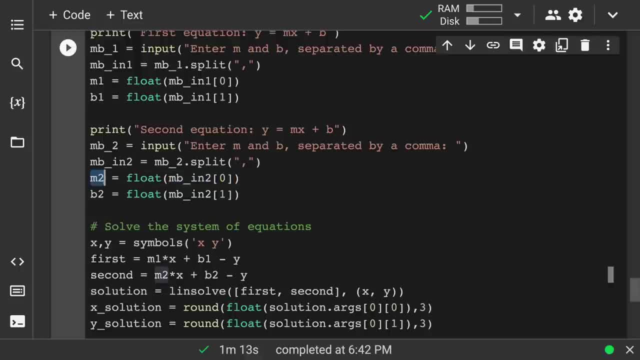 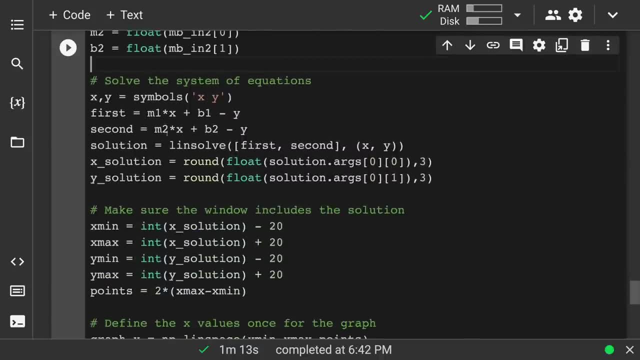 As A Float M Two. Second Element Cast As A Float B Two, And Now That I Have These I Can Solve It. So Here We're. 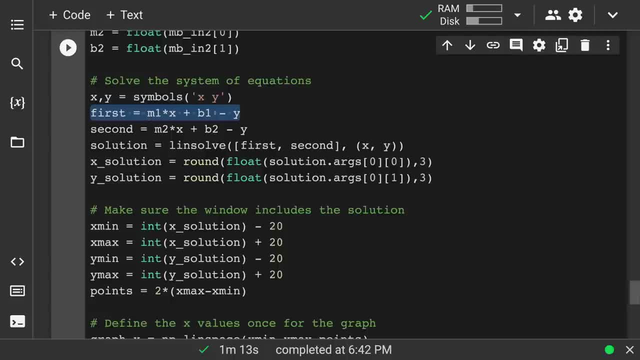 Using Sim Pie To Solve It. That Set To Zero. And Then There's The Second, And Then Lin Solve First, Second, And Then I'm Going. 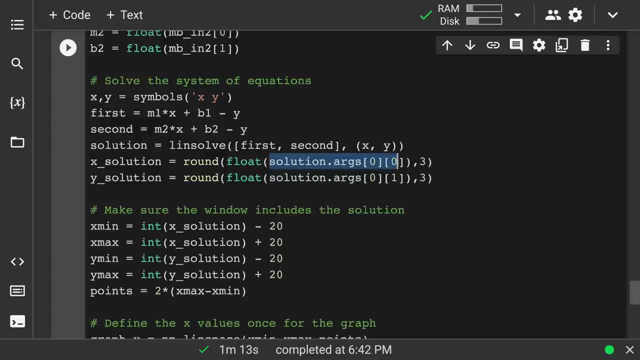 To, Just In Case There's Most, Just In Case There's A. So I Take That Solution Cast As A Float And Then Round It To. 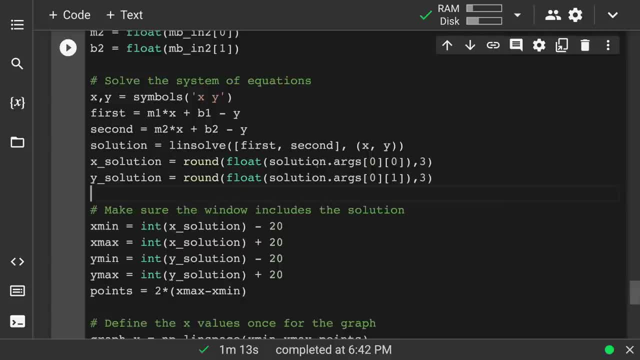 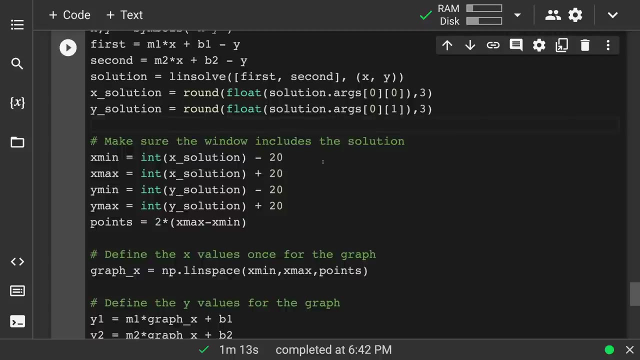 Three Decimal Places For Many Things. You Know, I Might Not Need It, But I Can. So Then To Make Sure The Window Includes It Rather. 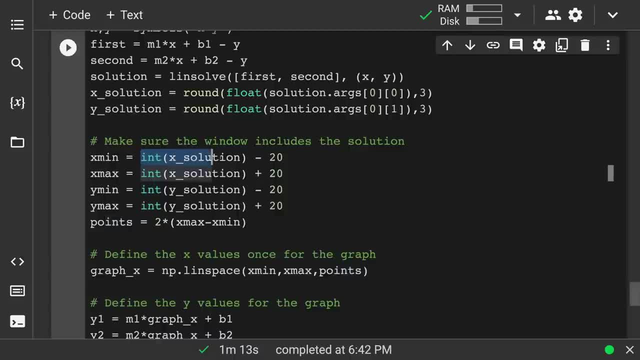 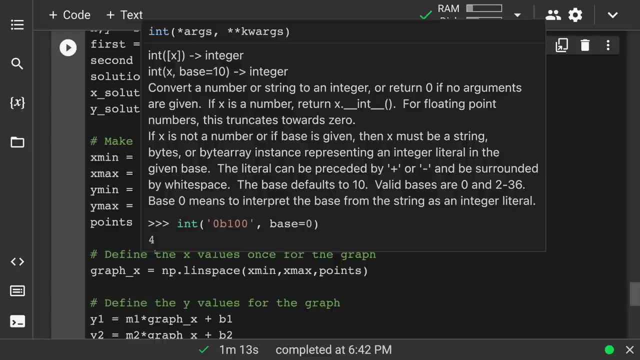 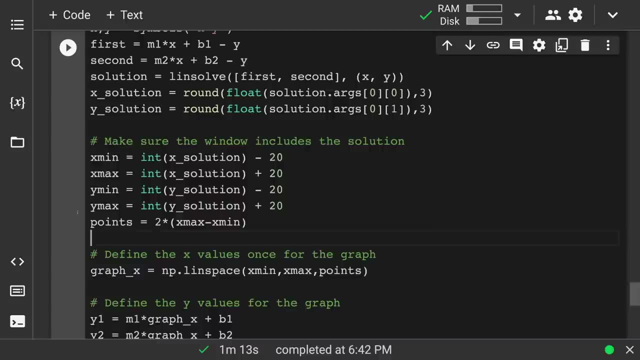 Than Give It To Be My Normal, My Normal Window, And This Is A Float. So If I, My Graph Is Going To Include That Solution. 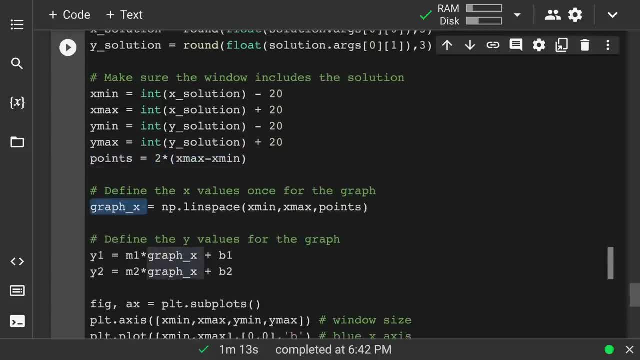 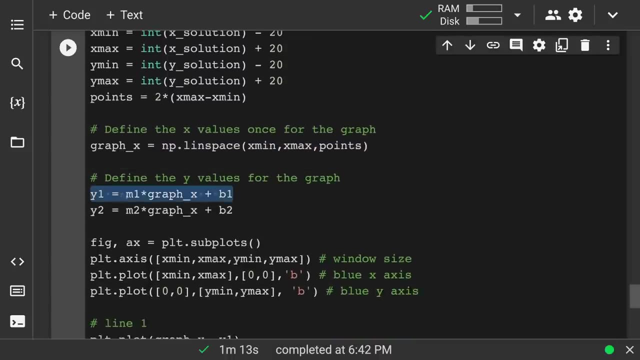 And Then Given These- You Know- Points, How Many Points Do I Want? And Then Graph X, Because I Already Used X And Everything Here For 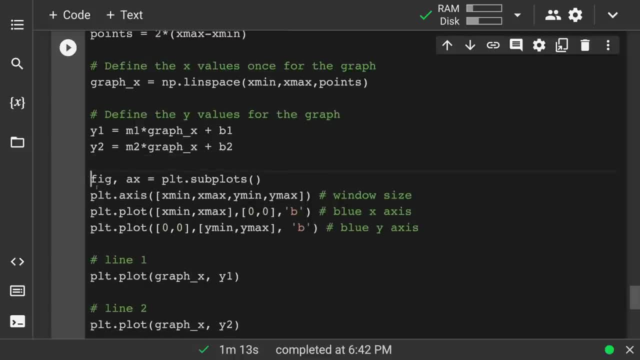 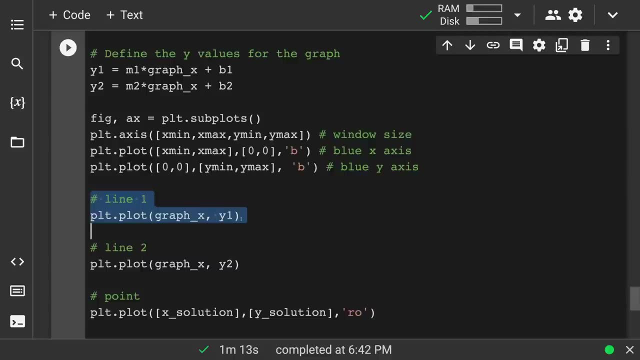 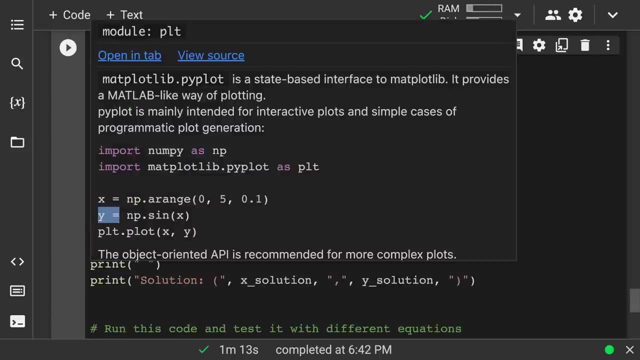 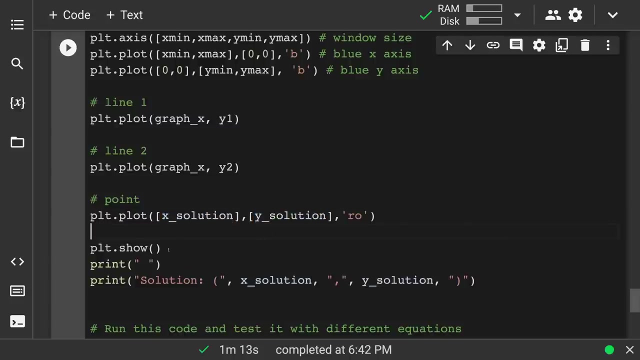 The Way To, Why? To M2.. Times Graph X Plus B2.. So Then, When We Set Up The Graph And Line One, You Graph X. 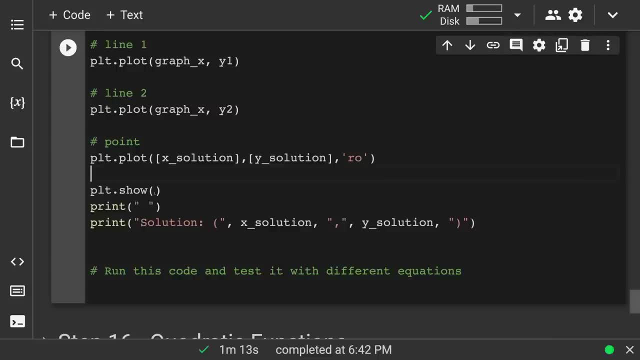 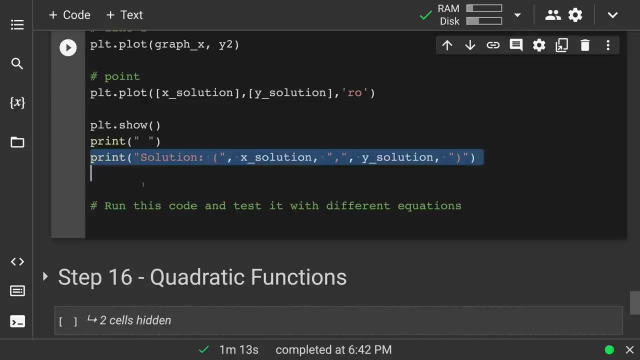 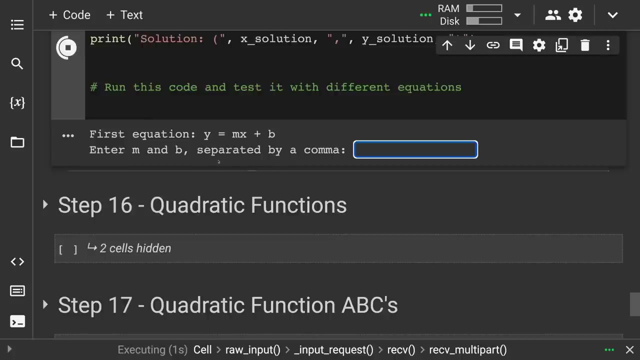 So That Way, Whatever Equations We Have, And Then Print Out The Value. So If We Take A Look At This, X Solution, Y Solution, 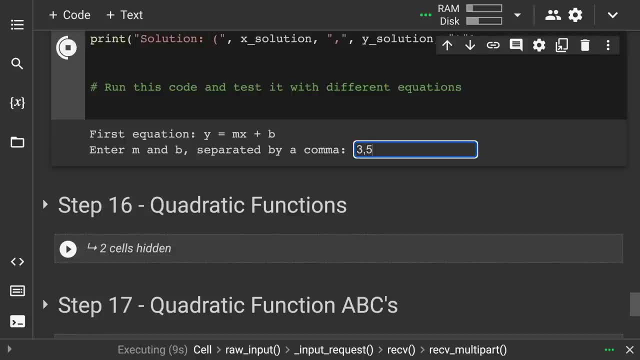 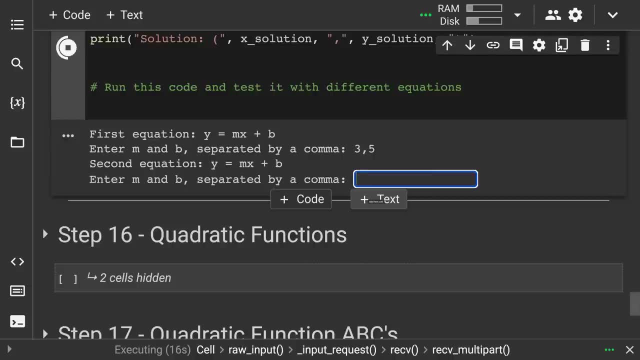 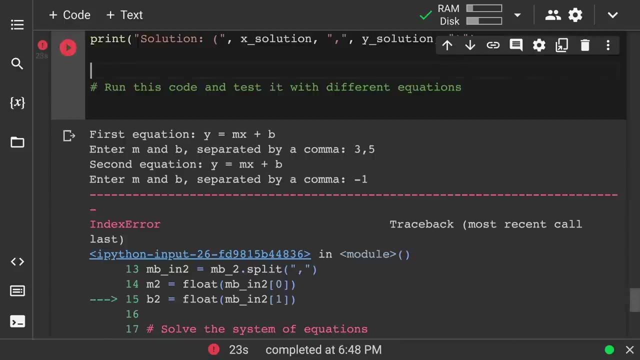 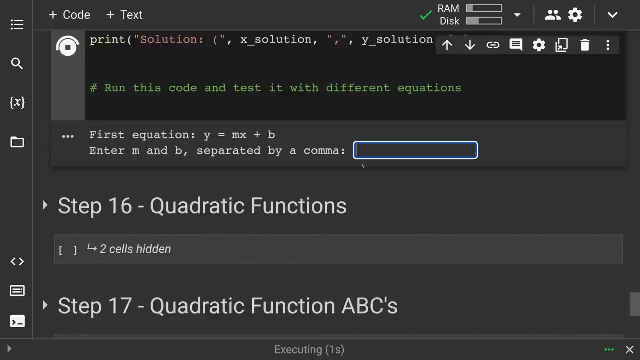 Let's See, Let's Call It Three, Five And Let's Call This One Um Negative One. Oh, Because I Didn't Put The Comma So. 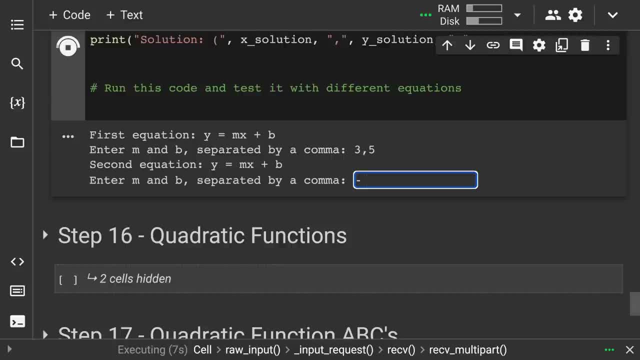 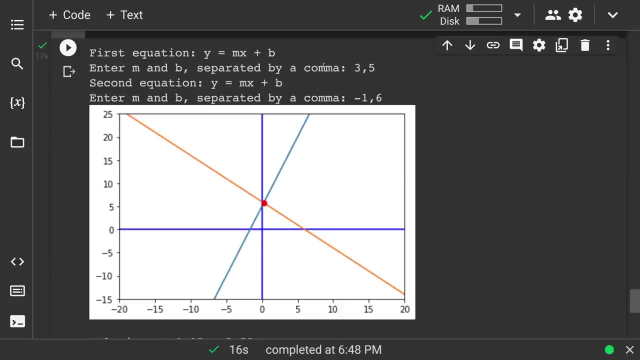 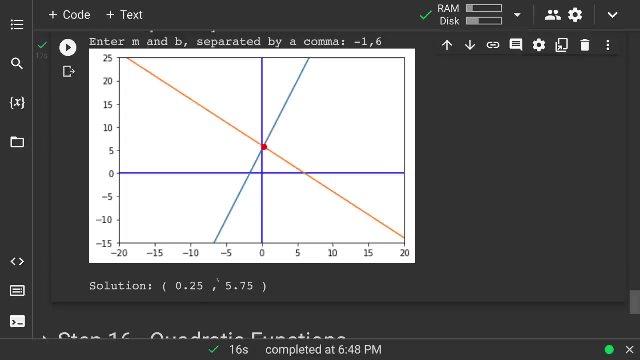 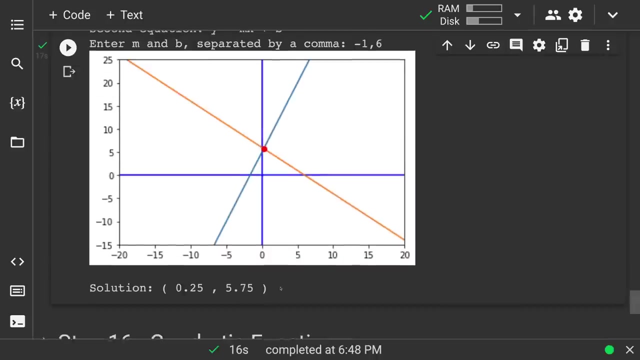 Three, Five And One, And There We Go Um Six. So We Have These And We See These Points. This Is The Solution, Even Though It 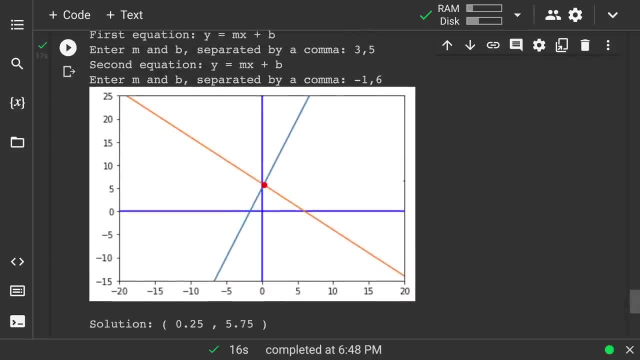 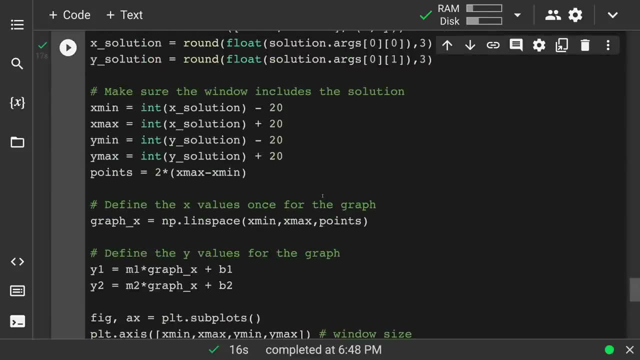 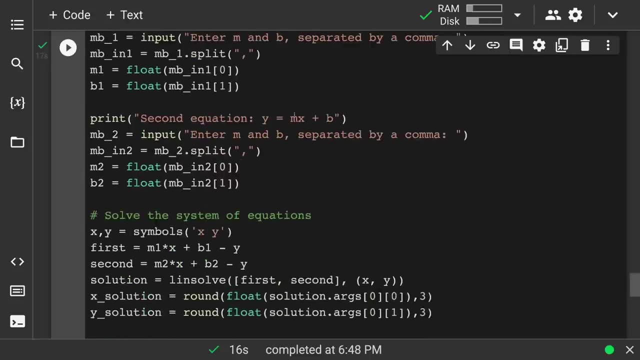 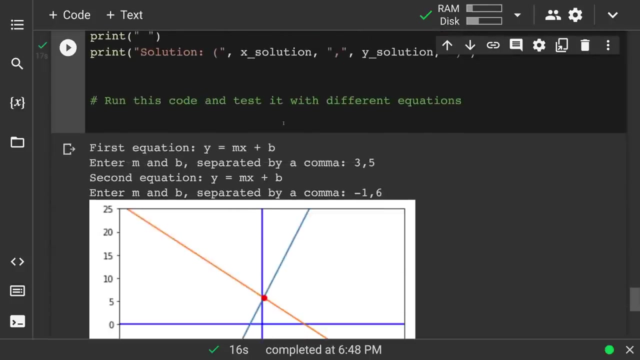 Is The Point Where They Intersect, And These Are Kind Of The Things That We Want To Build Upon. This Is Actually One Good Way. 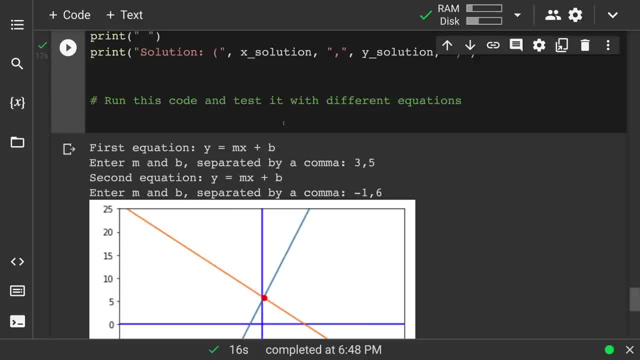 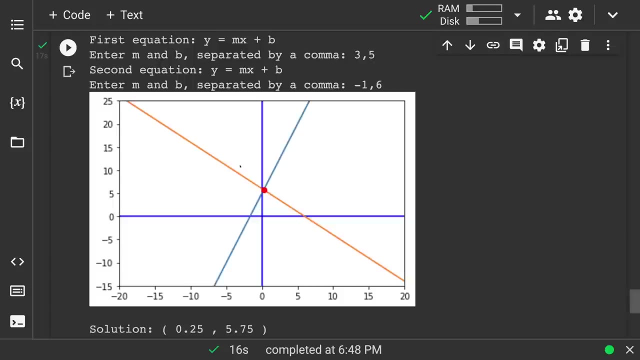 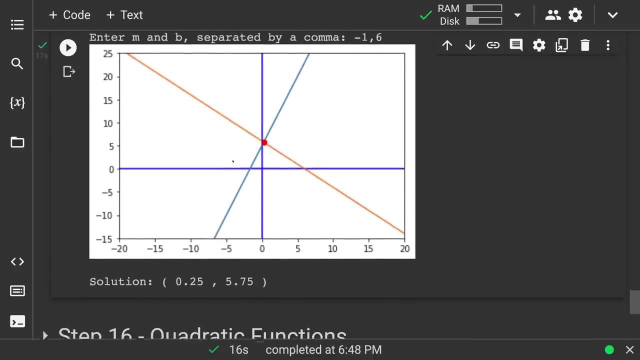 To Plot And Graph. Well, When We Get To All The Parent Graphs, All The Different Types Of Functions, You See That This Is One. 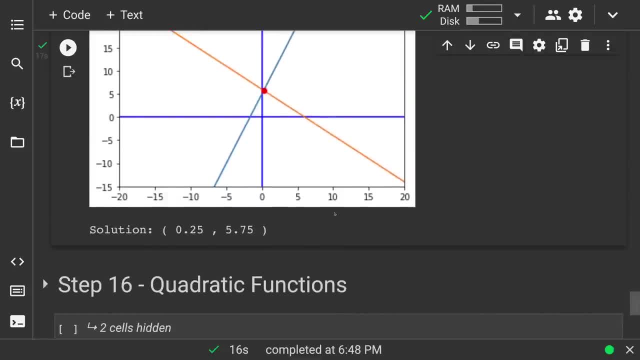 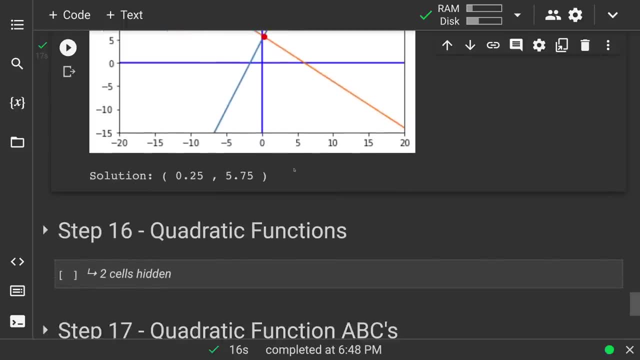 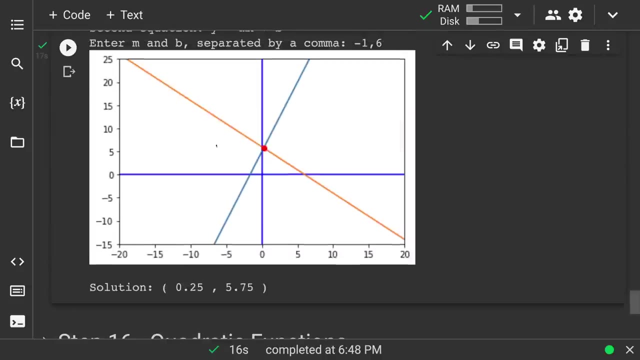 Way We Can Prompt, For You Know, If We Have The Next Thing We Have Is Quadratic Functions, When It's Not Linear Equation Anymore. 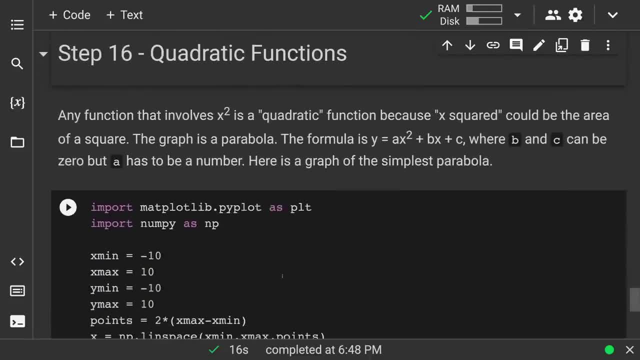 Not A Nice Straight Line. So Anything That Involves X Squared Is A Quadratic Measure Of The Side, But I Know That The Area 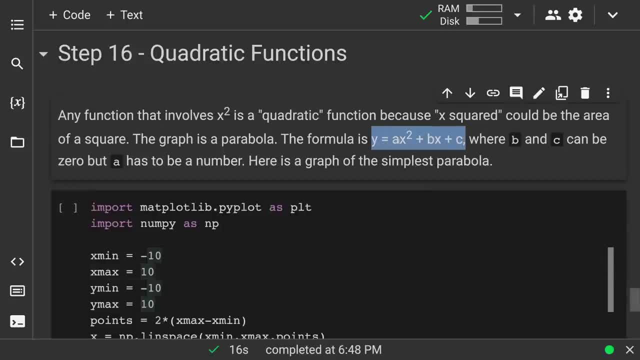 Would Be That Side Times Itself. So If I, If I Have X Squared In There, There's Going To, So Then You Know There's. 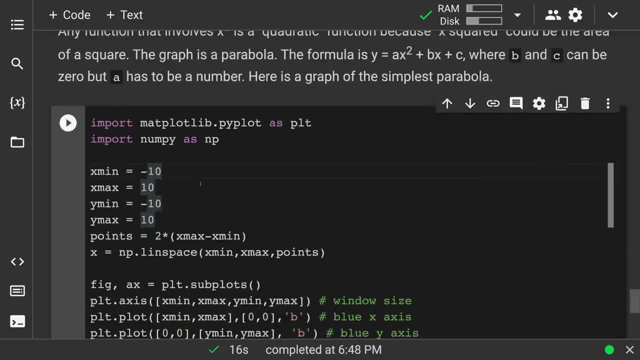 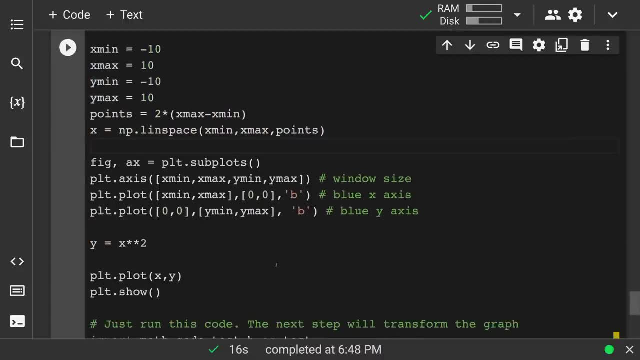 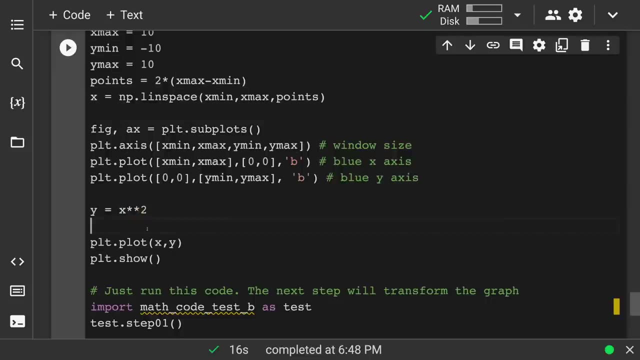 The Simplest One. So Now Let's Take A Look At This. Back To Our Graphing, Setting Up Our Points. You Know, Range Our Points. 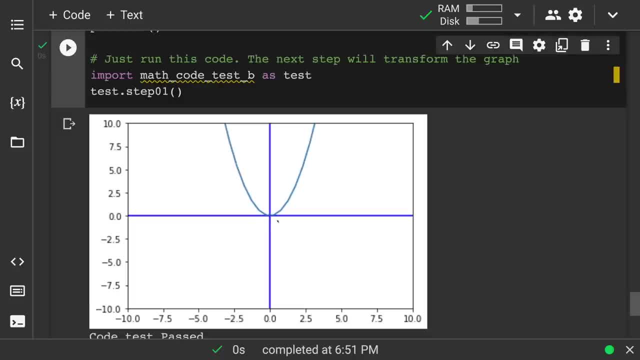 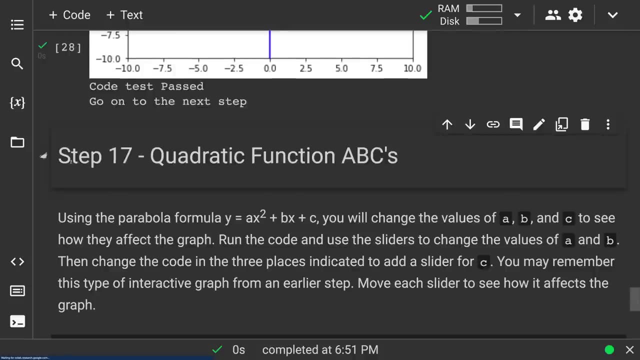 That's The Most Basic Parabola, So A In That Case Would Be One, And You See It Does Touch At Zero, Zero, All Right. 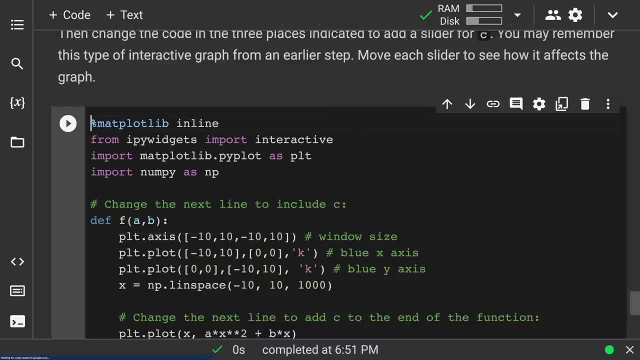 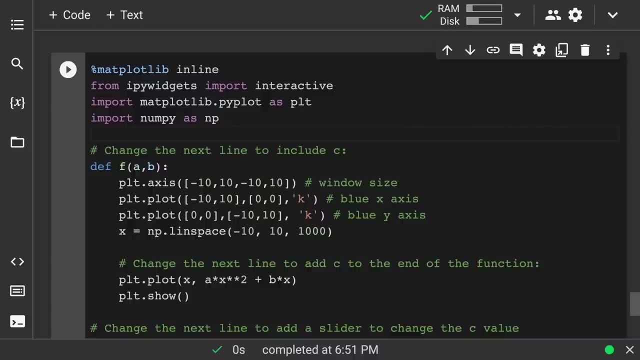 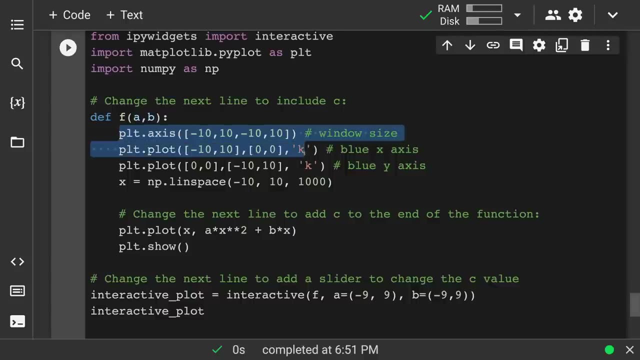 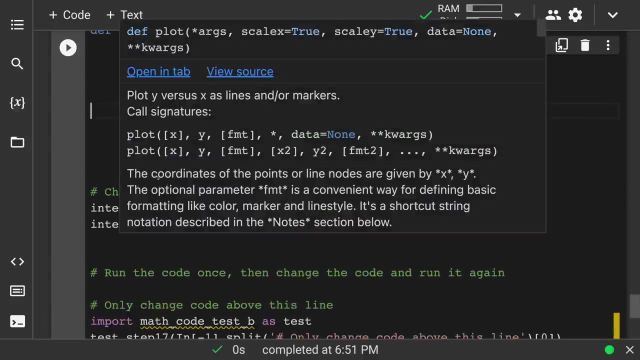 The Most Basic Parabola, So This One Here. All Right, You Have A And B, But We Forgot C And We Could Have Also Put. 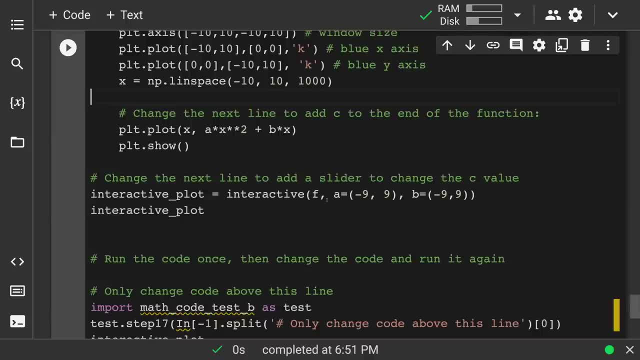 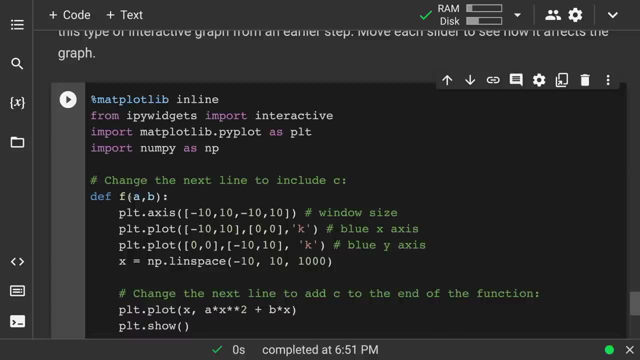 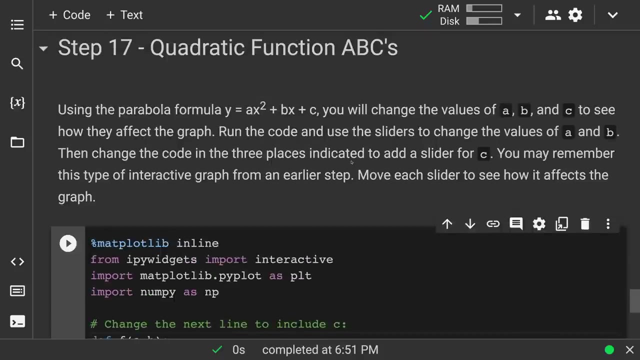 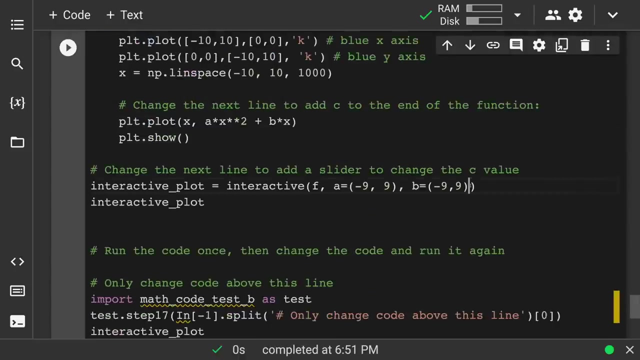 The Values On. You Know In A Different Way, But We See Function Here- A, B. But I Want A, B And C, So That's. 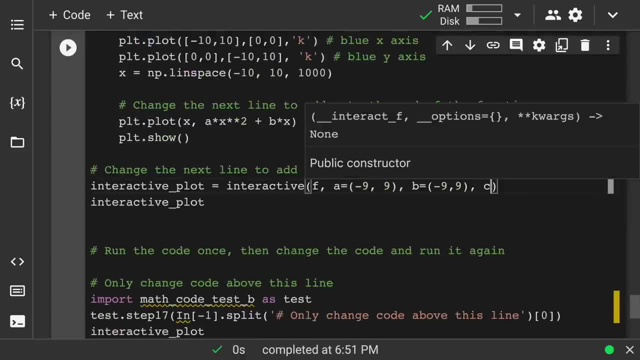 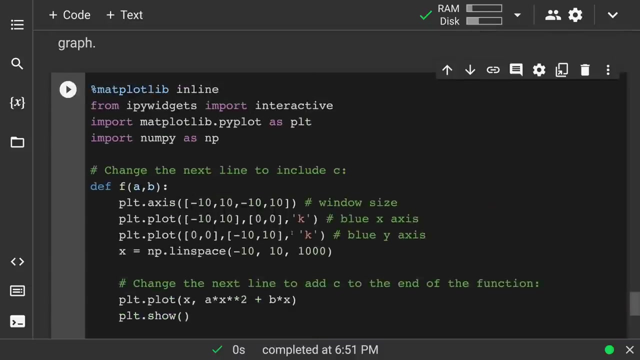 Going To Be Your Assignment. Add C To The Slider. So There We Go, Out, There We Go. So Now I Have This Interactive, I'm 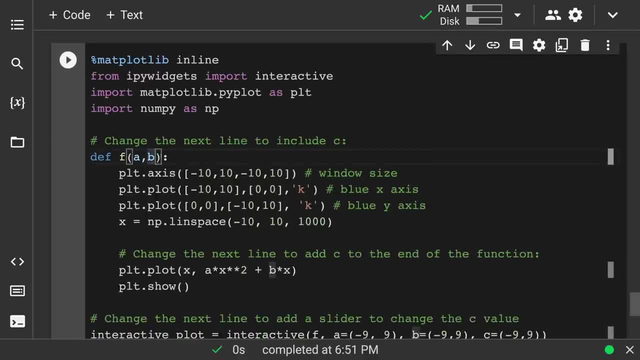 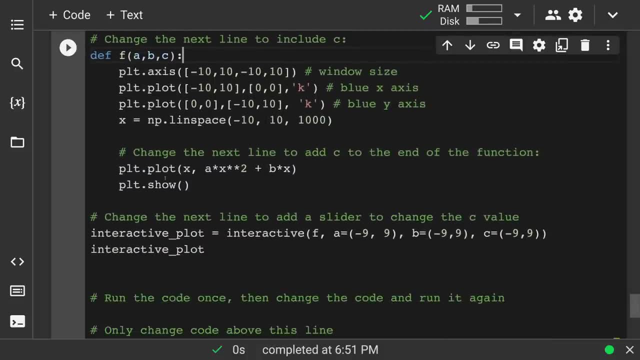 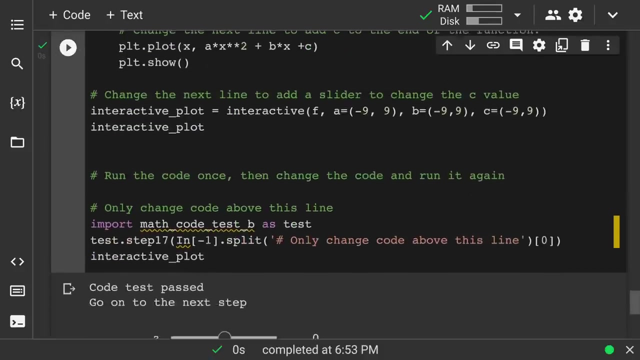 Going To Have Three Sliders: One For A, One For B, One For C, And Then When We Define A. So Now, When We Run, 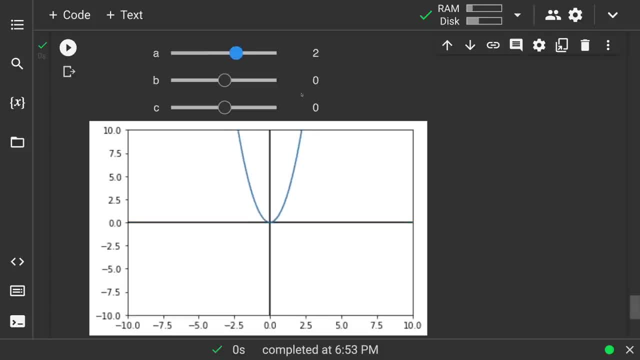 It Now It's All Zeros. That Doesn't Look Like Anything, But As Soon As A Is Something. Now We Don't Have A Parabola. 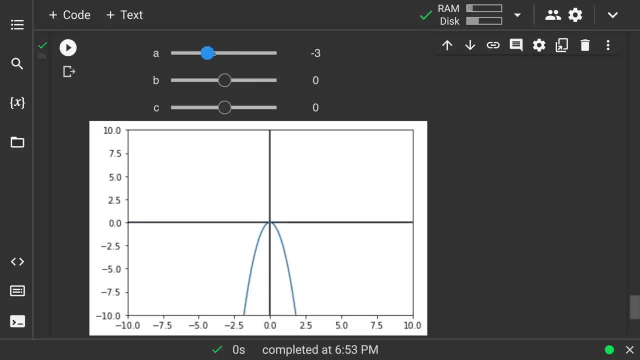 But Negative Values. It Flips It So: Positive Like A Smile, Negative Like A Frown, And There We Go. So Let's Have A Positive. 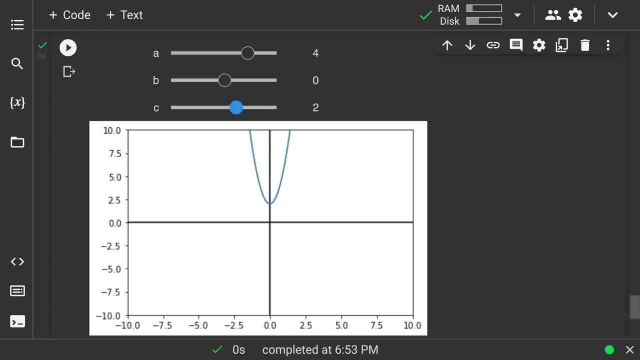 So We're Down And Could Be Zero, That's Fine, It Just Touches Zero, Zero. So That's What C Does. It Moves It Up, Or? 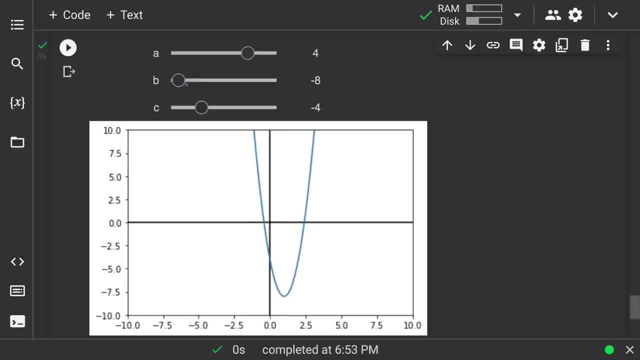 Down The Y Axis And Then B Is Very Negative. But Now When B? If B Is Zero, It's Symmetrical On The Y Axis. But 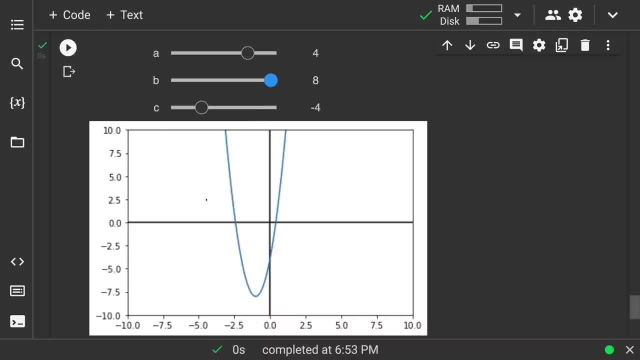 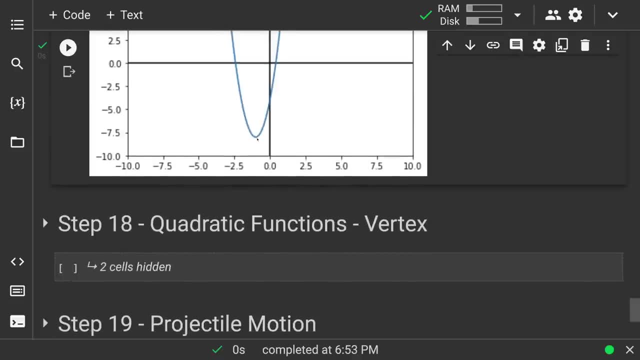 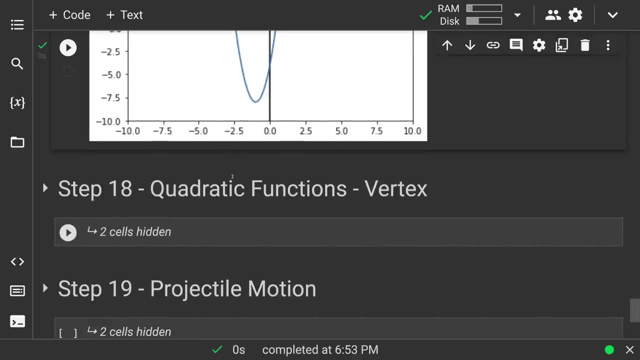 Then It Goes Around And Then Now Positive B Value Stretches On This Bottom Part, Or If It's Flipped Over, That'd Be The. 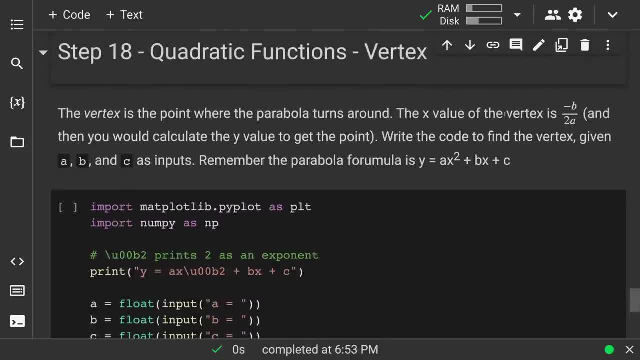 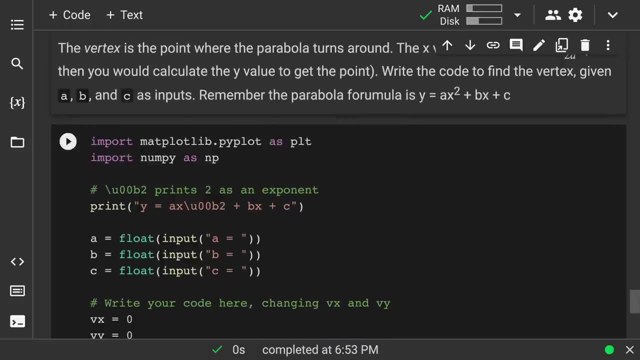 Top Part Where The Turnaround Happens. That's The Vertex. So That's The Point Where The Parabola Turns Around And We're Going To. 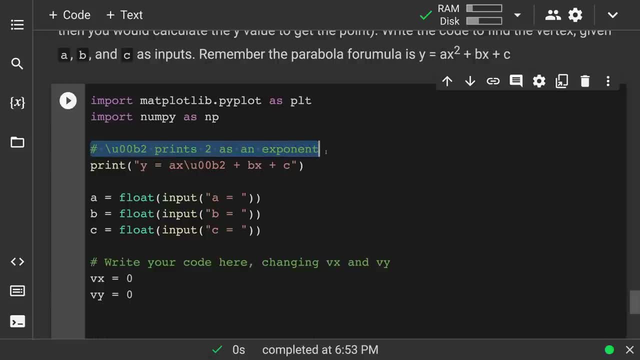 Create The Parabola. Now This: I Even Have The Comment Here Because Certainly I Can Print X With The Two Asterisks For The Exponent. 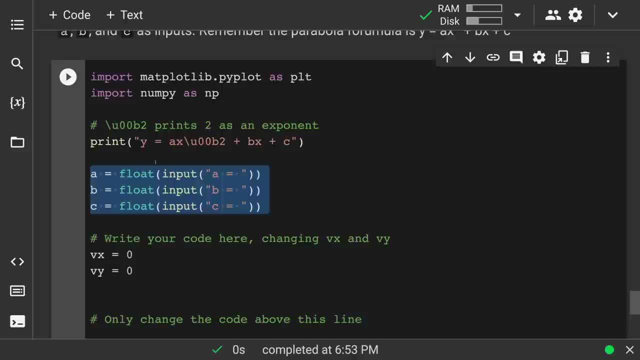 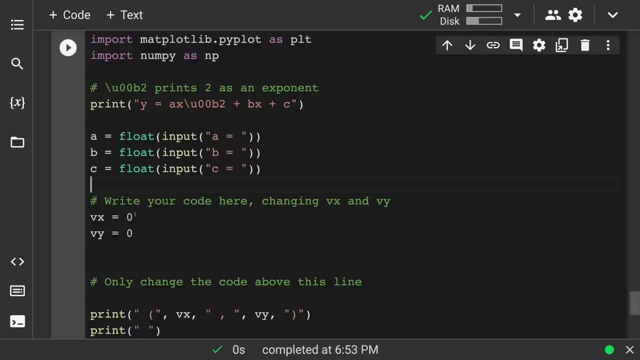 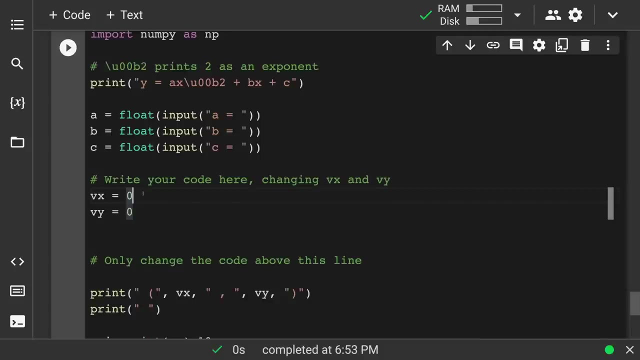 But We Know, We Know We're Doing A Parabola, So We Just Prompt For These Input Values. All Right, Then What Would Be The? 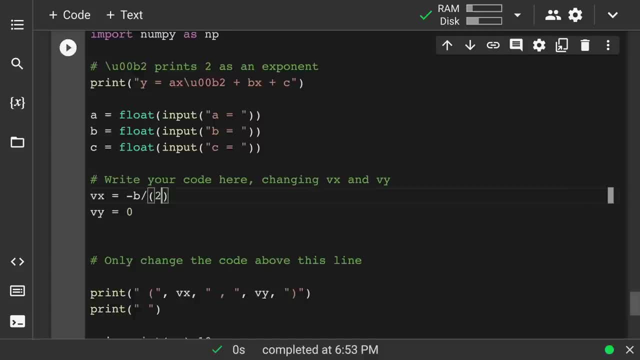 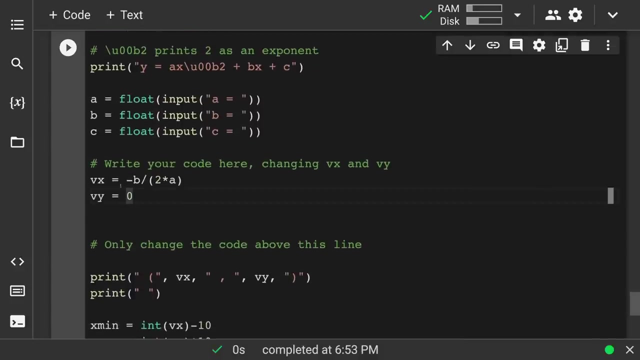 Vertex. Well, The X Value Was So Negative B Over Two A, Because If I Don't, It'll Divide By Two, Then Multiply By A Doing. 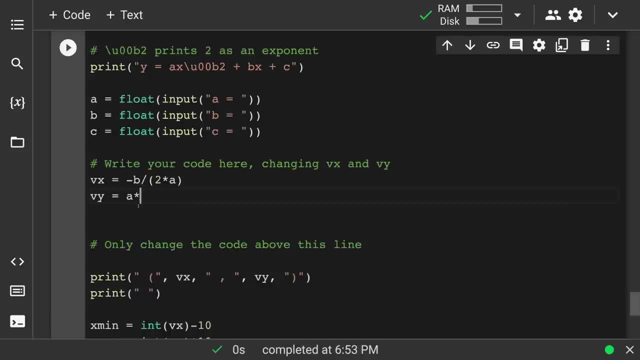 Order Of Operations. Now, If I Have That Value, Then A Square Plus B X, So To Be V X, Because I Want The X Value. 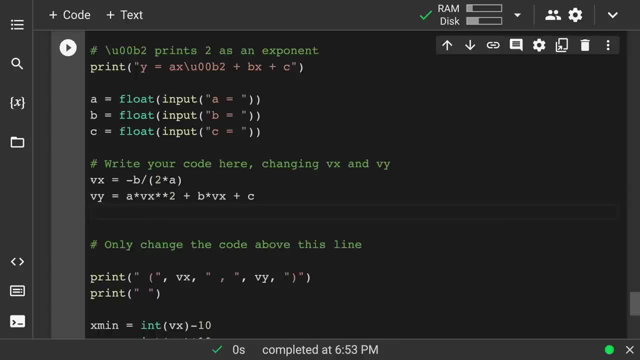 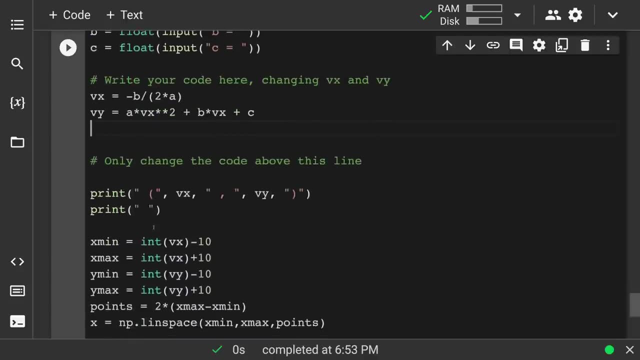 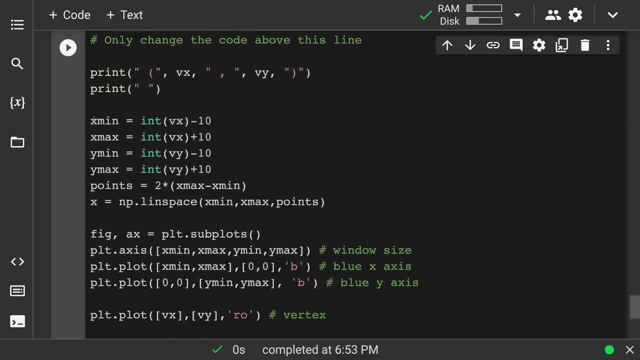 Of The Vertex Plus C. So There We Go. So I Use This A And Then X Minimum. So For Whatever We Enter, We'll Just 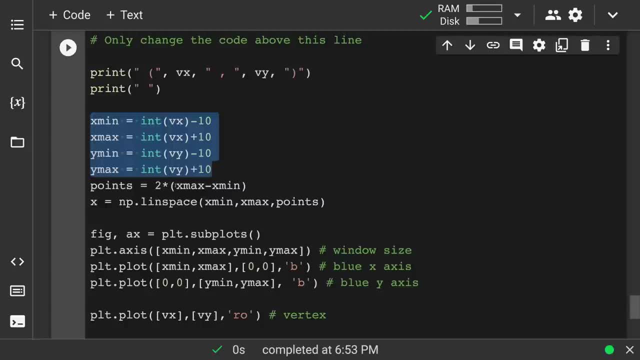 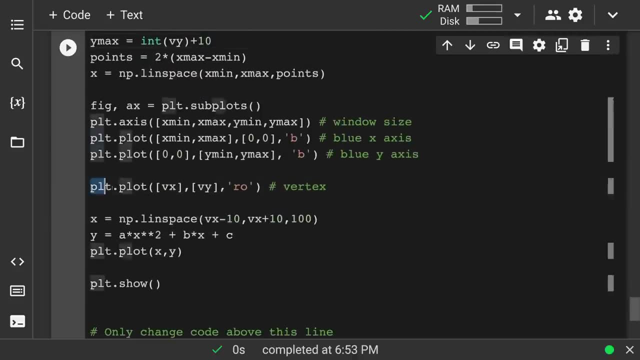 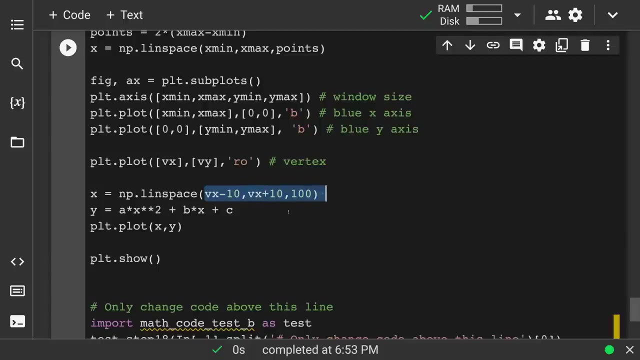 Make Sure That That Does Show Up On The Graph. So Counting Whatever These Values Are, And I Probably Could Have Done This Based On 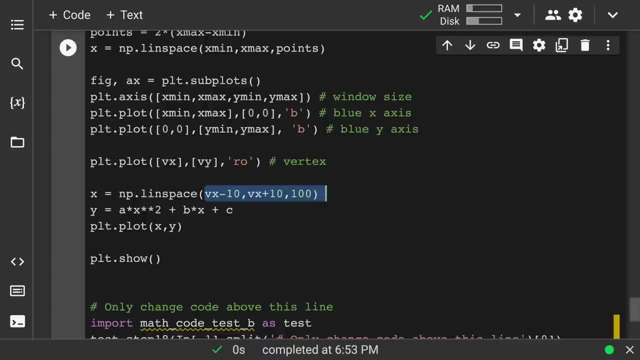 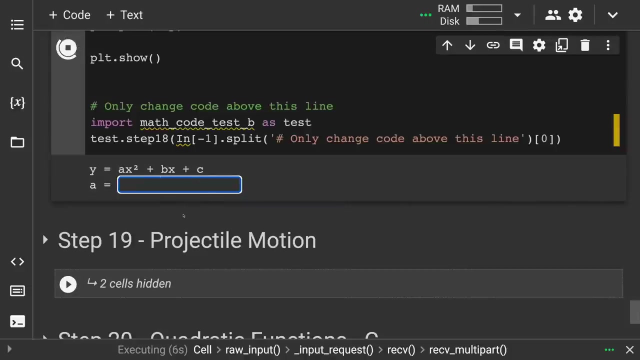 X Min, X Max, But Just Doing This Anyway. Notice The Lens Space, Just Giving Us That Enough Before And After. You See, That's A. 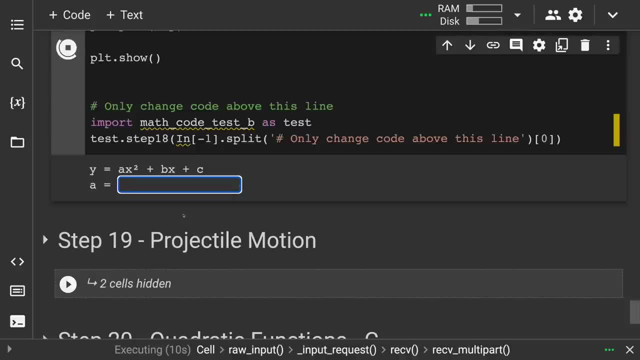 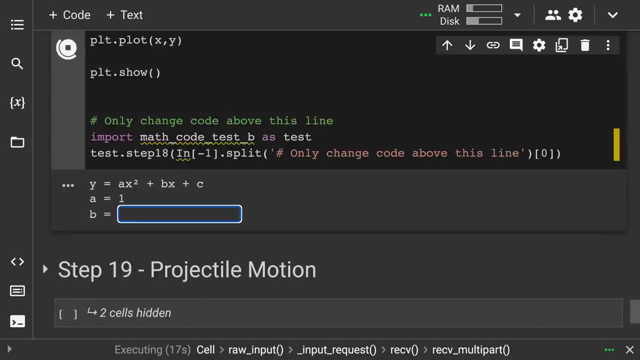 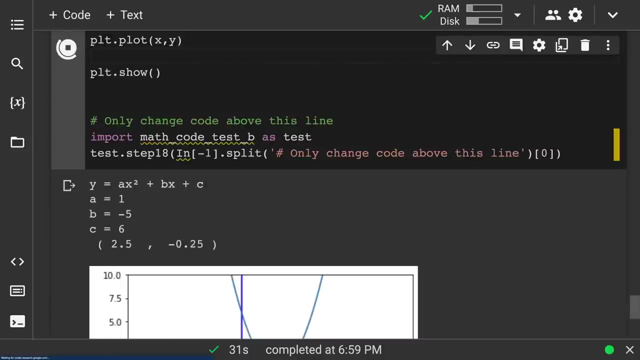 X Square. You See That Little Two. That Was The Whole Idea To Get To Be That Fancy. So A X Square, Let's Just Try. 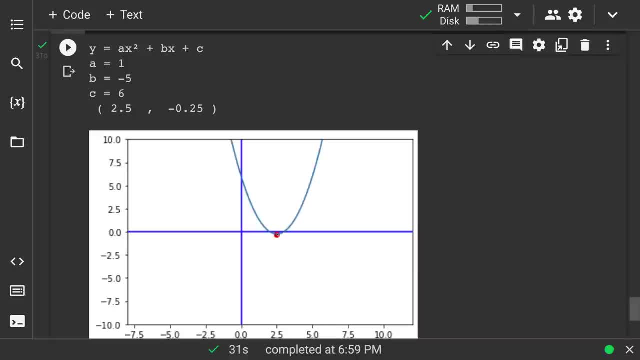 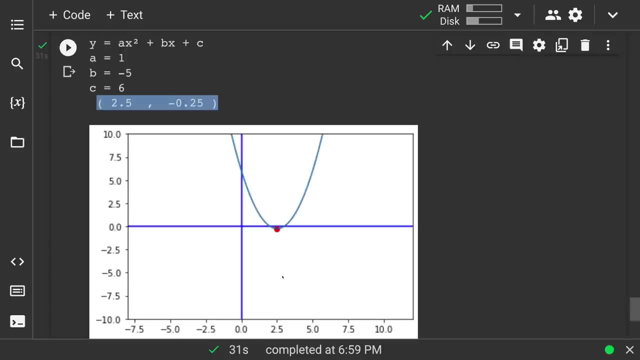 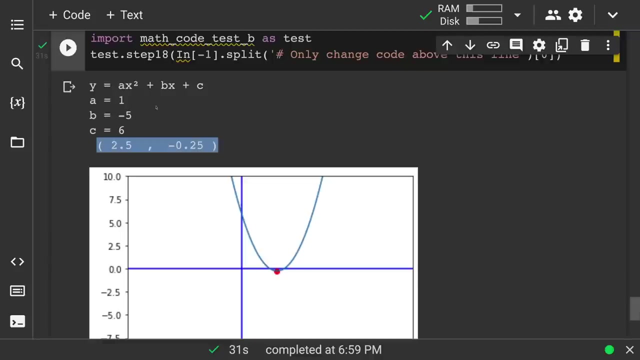 So We See The Vertex, And The Vertex Is Two Point Five Negative Point Two Five. And We See The Parabola, And Then We See: 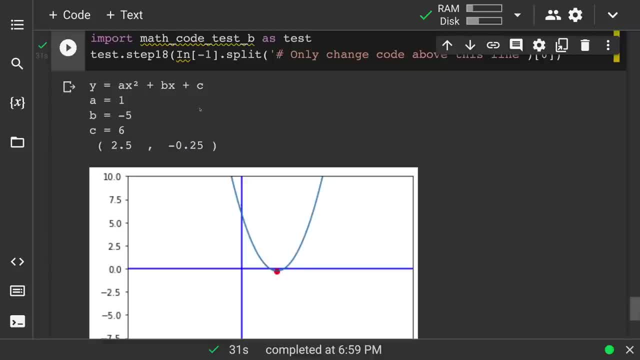 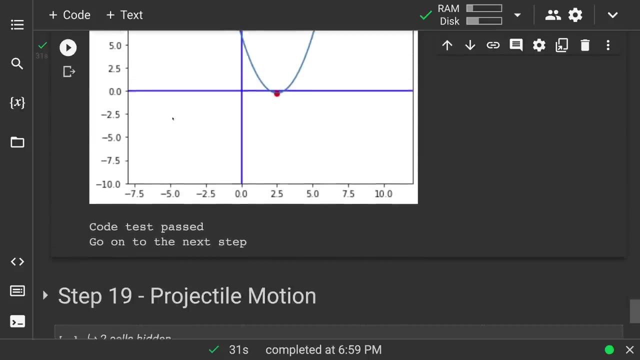 The Vertex Plotted, So Did The Linear Equation Plotted For M And B. We Can Do A Quadratic And Plot For A, B And 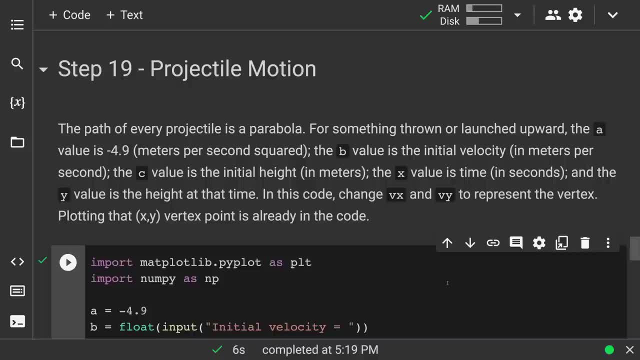 C. So You Know, We Could, We Could Do, And They All Actually Make The Path Of The Parabola Pretty Interesting. It Can't Not. 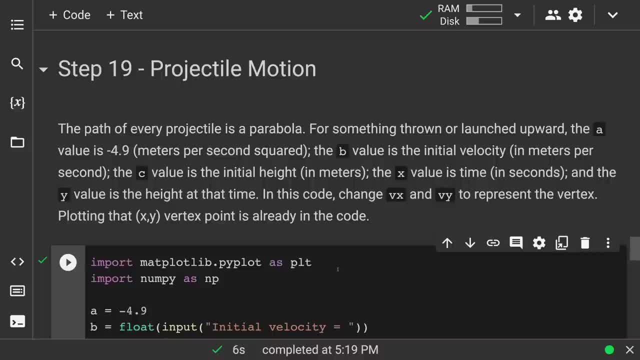 Be A Parabola. So As We Look At These, The Path Of Every Projectile In The World, So We Know That The A Value Stays. 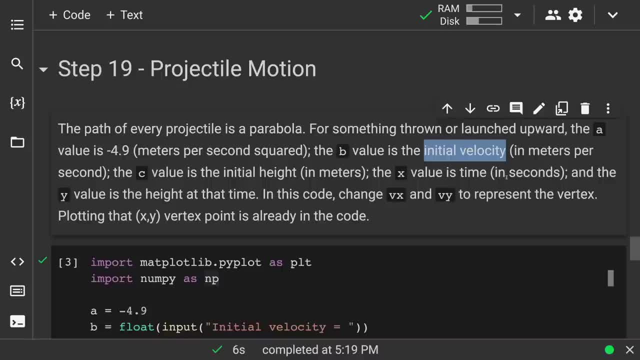 The Same. The B Value Represents The Initial Velocity, So That'll Change Depending On How Hard You Throw. You Know The Path Of The Ball. 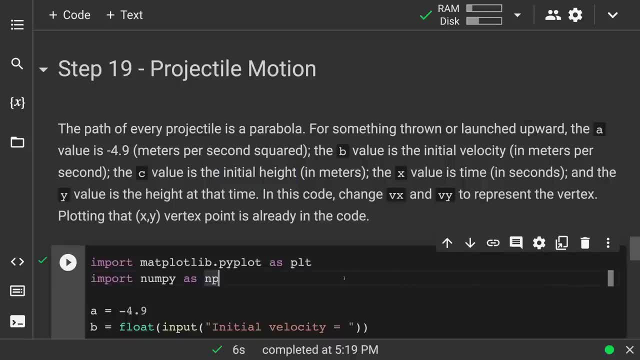 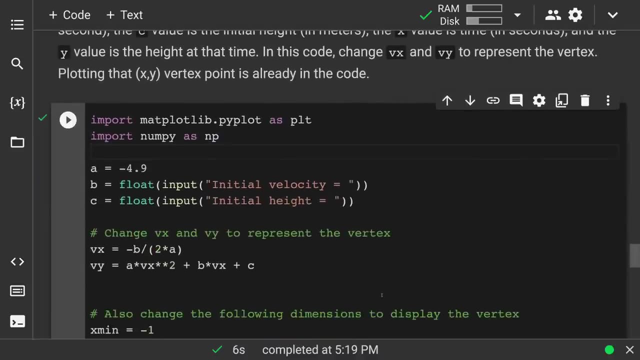 Is A Parabola, And Then In That Case C Would Be Zero, The Initial Height In Meters. So We Have Our Classic Negative Four. 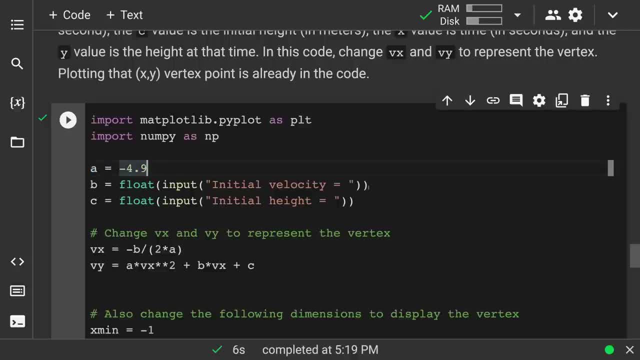 Point Nine. So I Don't Even Need To Prompt For That. If It's A Projectile That's Going To Stay The Same, The Initial Velocity. 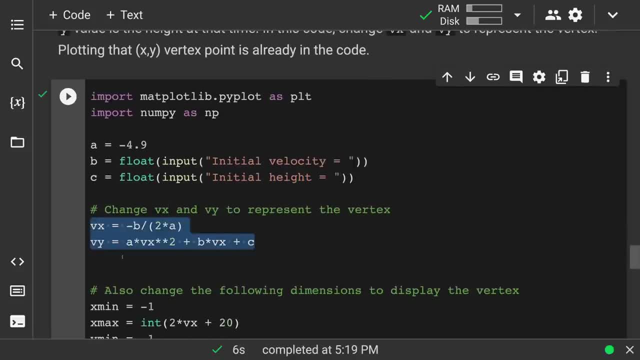 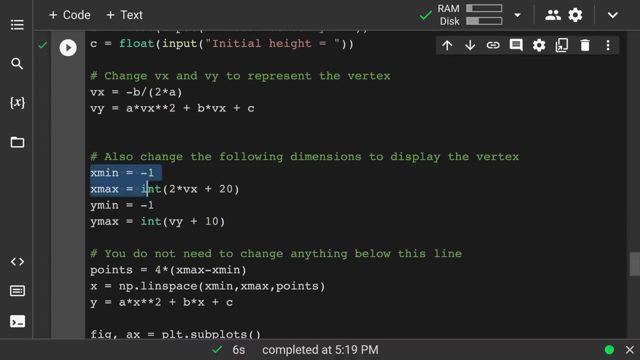 I'm Going To See The V X And V Y Code From The Last Step, Because The Equations For The Vertex Are Exactly The Same. 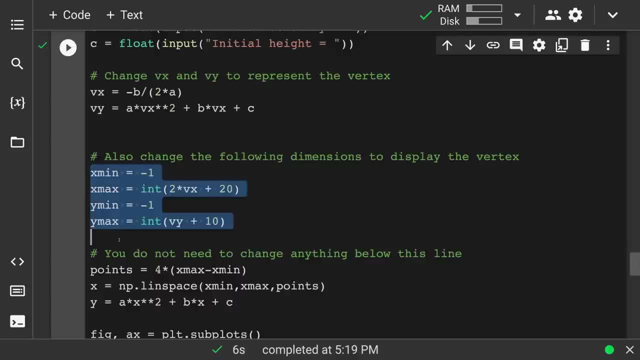 So You Know, Once We Have These, But Really We Just Are Going To Be Concerned About Positive Values Here, So I Made X Min. 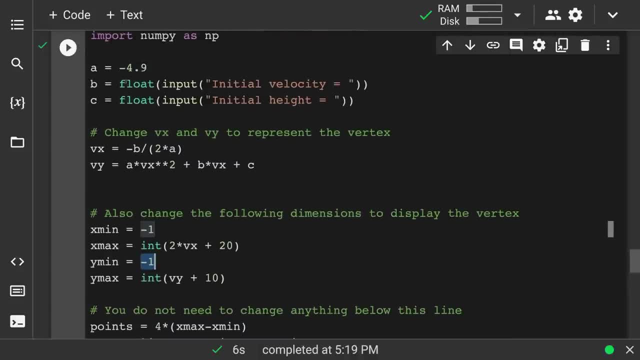 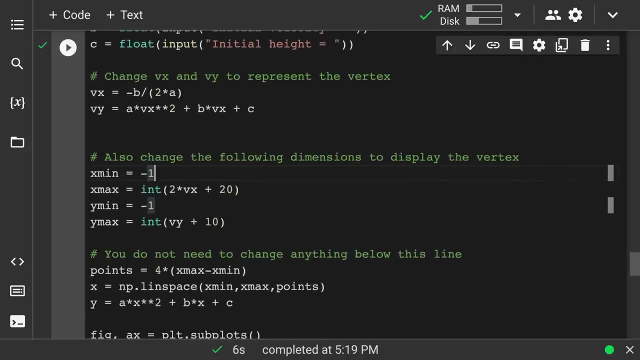 Negative One, Just That Little Bit Negative To, So That You, I'll Tell You This, All These Parabolas Are Symmetrical, So The X Value 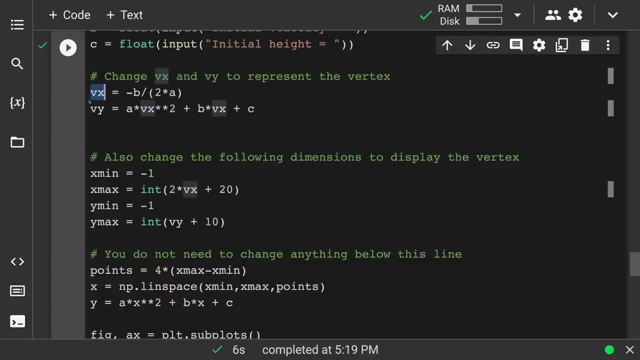 The Vertex Is Exactly Right Down The Middle. Sometimes We Call It The Line Of Symmetry 20.. Just To Be Sure We See The End. 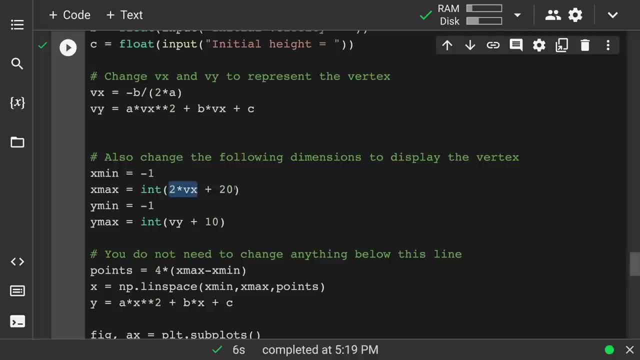 Of It To You Know, And Maybe A Little Bit More. It Gives A Good Perspective On The Graph. So The Vertex That's Going To. 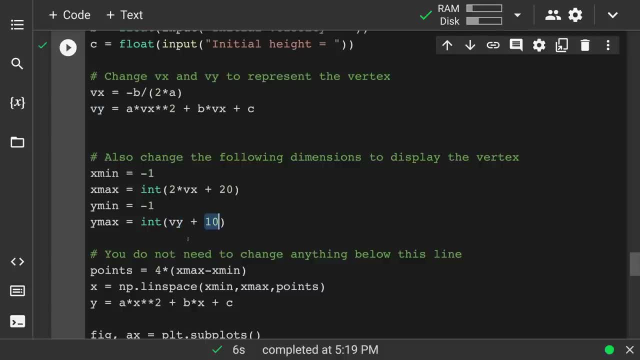 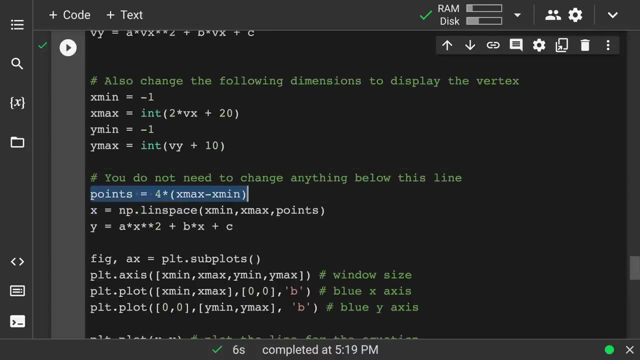 Be The Highest Point Of Our Projectile, And I'm Just Going To Add 10. To It. I Figure That's Plenty, Just Enough, So That. 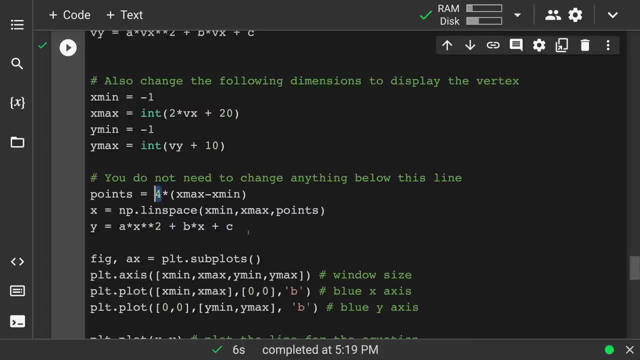 Just Just In Case, To Make Sure Our Graph Isn't Choppy To. Might Even Have Been Enough, But There We Define The X Values Same. 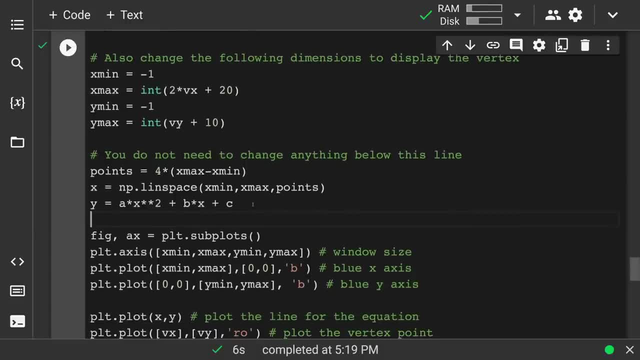 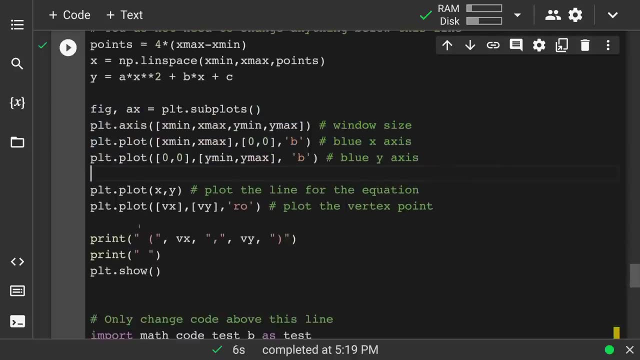 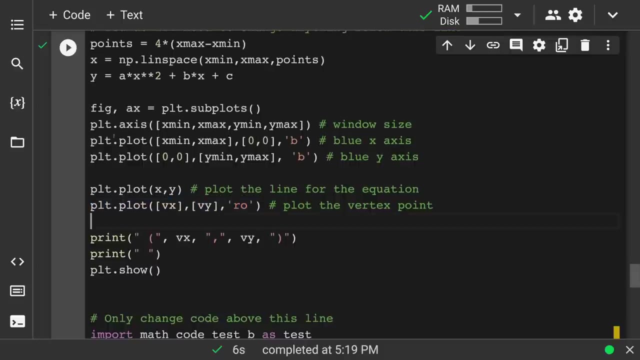 Function We Been Using. Now We're Going To Plot That Same Stuff. We've Been Doing Plot, And Then We're Also Going To Plot You. 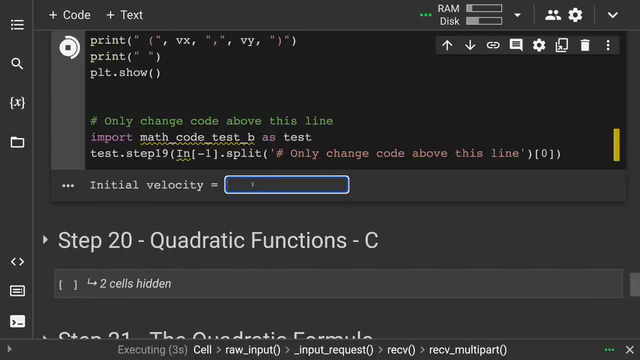 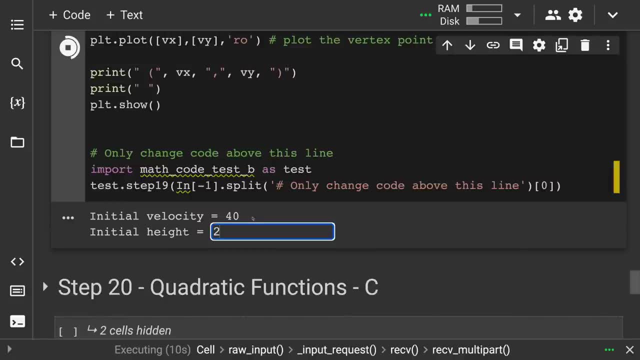 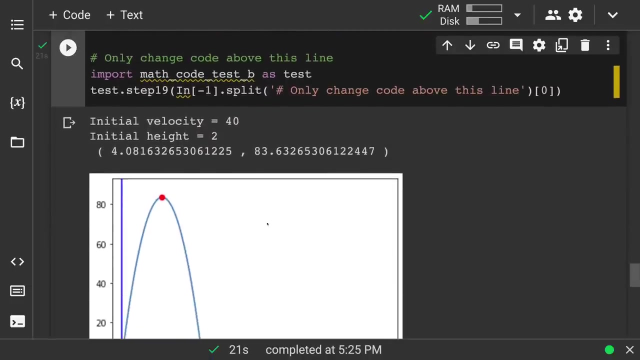 Know A Red Dot For The Vertex And Display. So This Could Be Something Like A Baseball That You Throw Up In The Air, You Know. 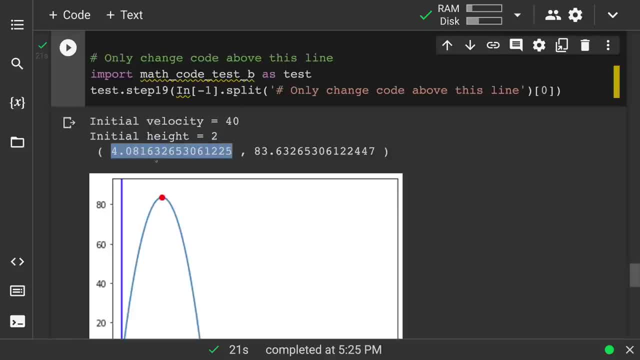 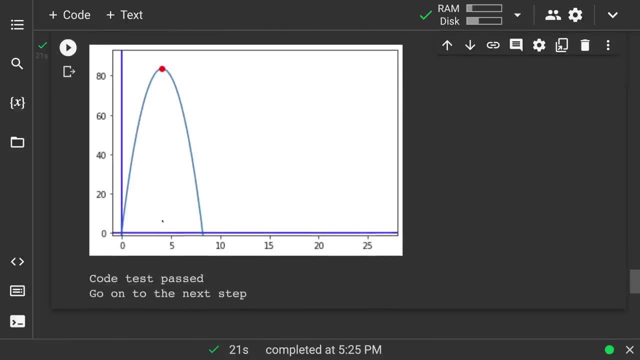 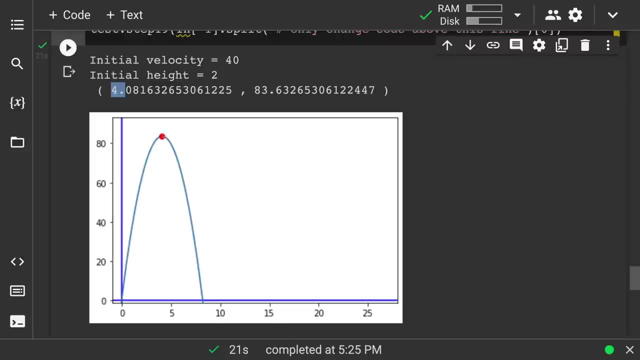 You Could Probably Throw It At 40. Meters Per Second Straight Up Time. Is That Just Over Four Seconds After You Throw The Ball Up? 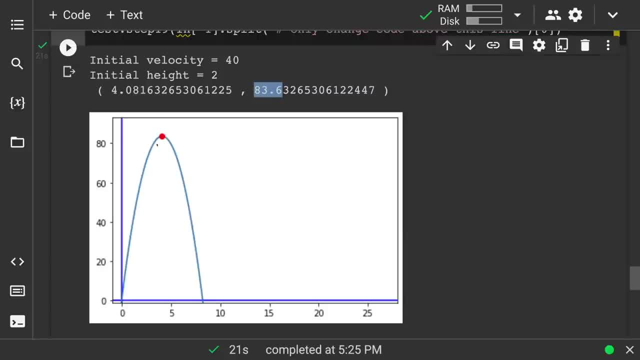 In The Air. It Will Hit Its Maximum Height Of A Little More Than 83. Meters In The Air, And Then Time Wise, You Know. 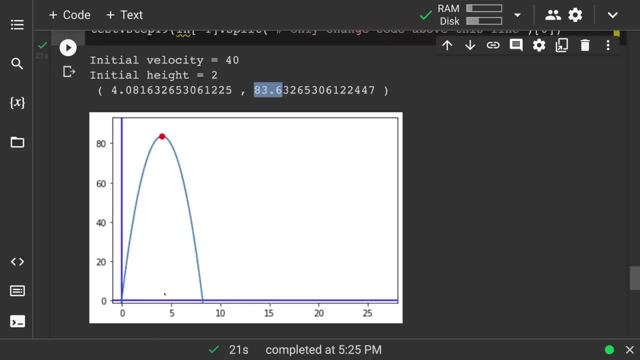 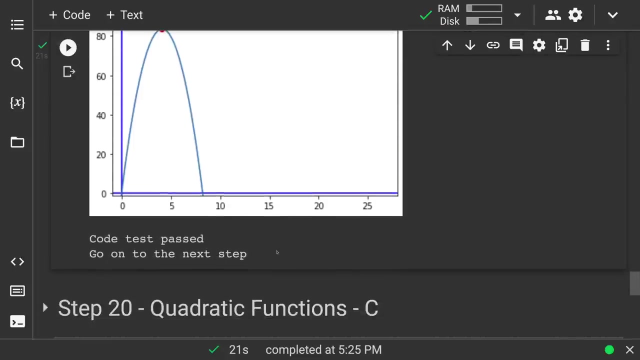 Four Seconds Or So In Is Good Where It's Going To Hit Its Highest Point And Then Little More Than It Will Be Ball Thrown. 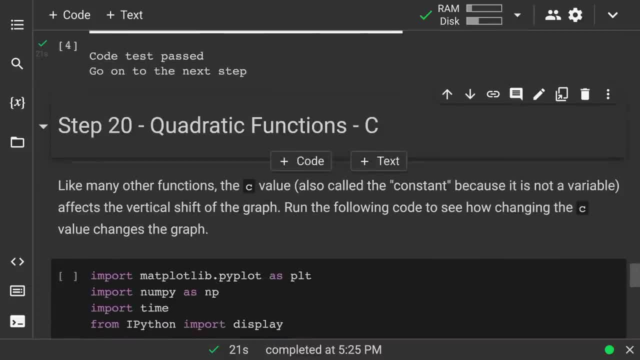 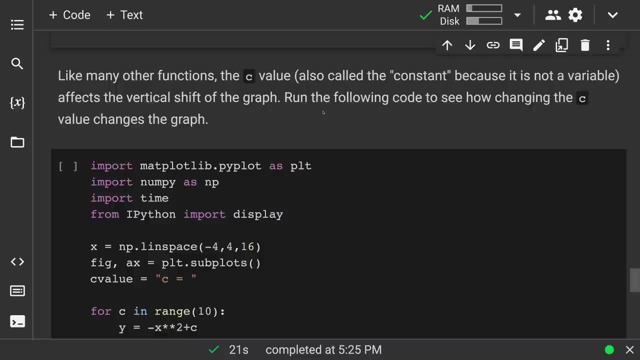 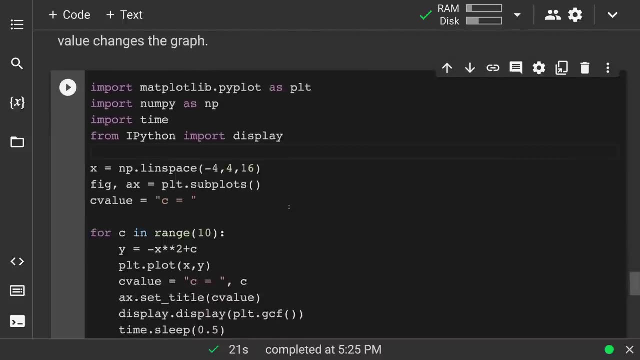 Or Rocket Launched. Yep, There We Go. So See, I Just Broke This Out, As You Know. See If Everything Else Stays The Same. 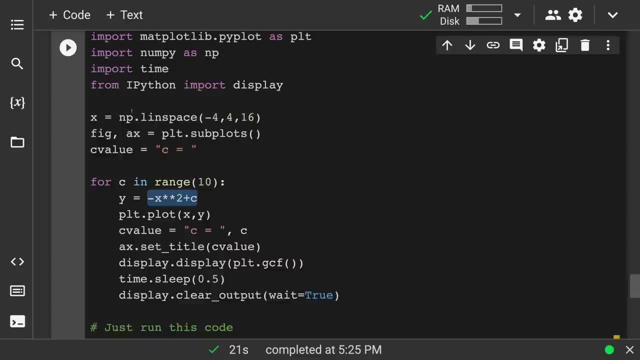 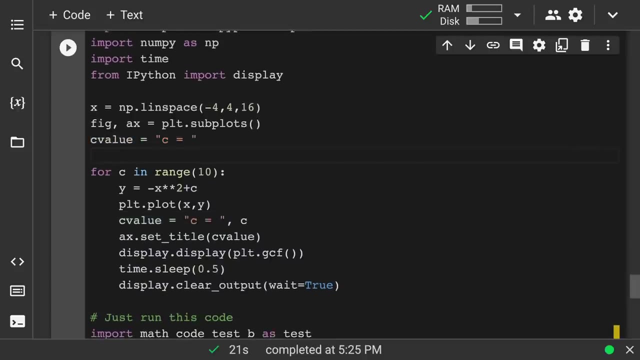 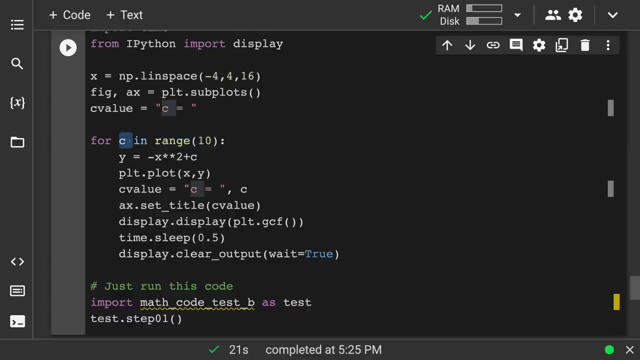 Negative. So We Take A Look Our X Values And Then We Plot. We Decided To Make Create This C Value, C Equals And If 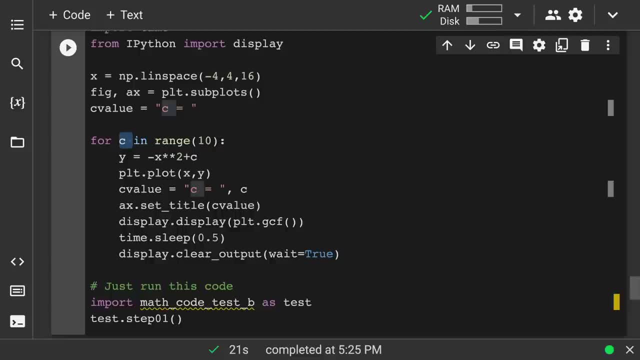 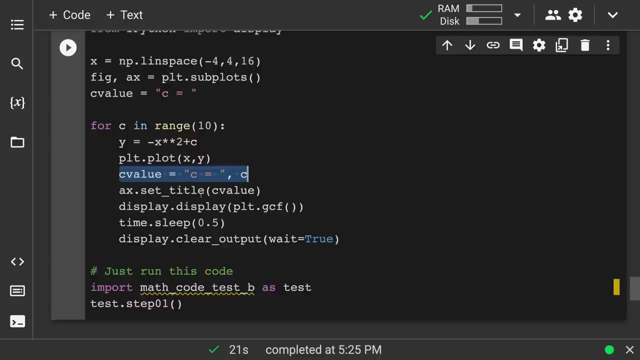 We Take A Look. So Then I Made It Negative: X Squared Plus C. And Then What Are We Going To Do? We're Going To 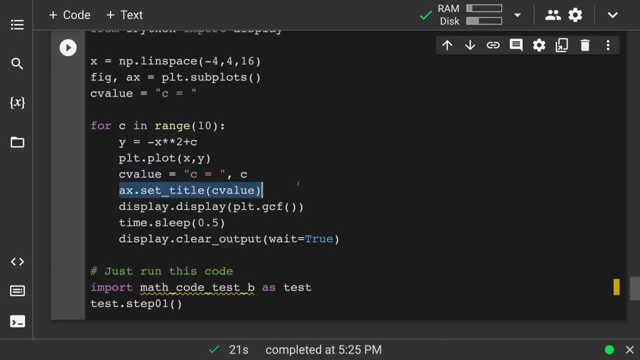 Plot It To Find The X Values. Once Up And We're Going To Display And This Little, This Little Display Here You, You'll See How. 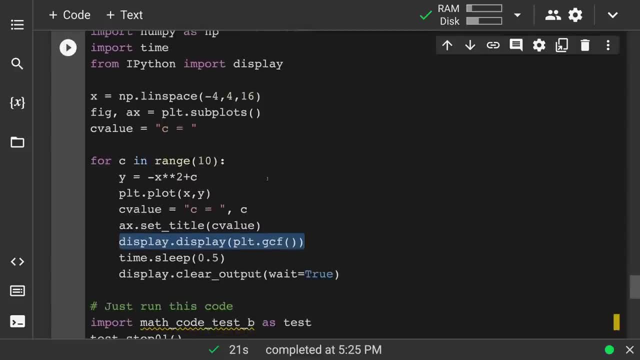 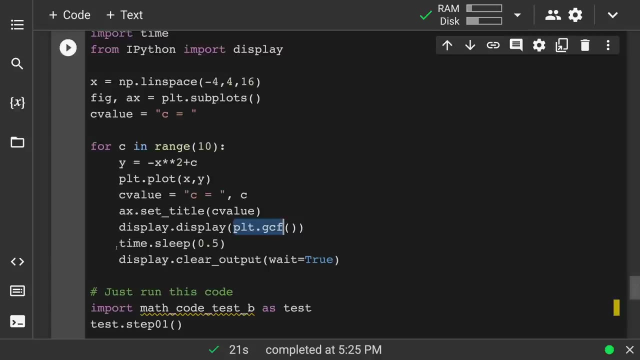 That Just Makes It Play Out The Notice. I Don't Have The Defining X Graph Fit, And Each Time. So Here's A Python Sleep. 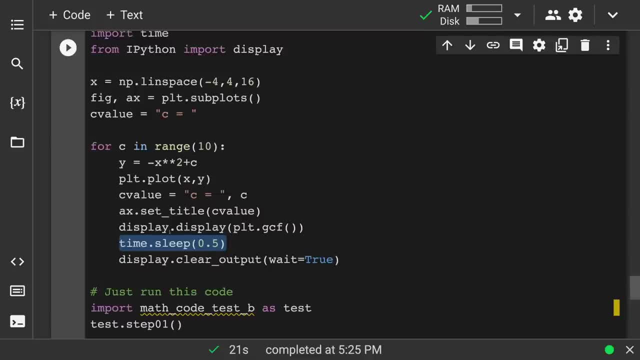 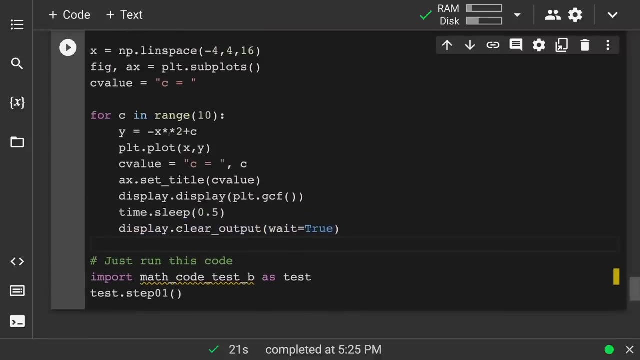 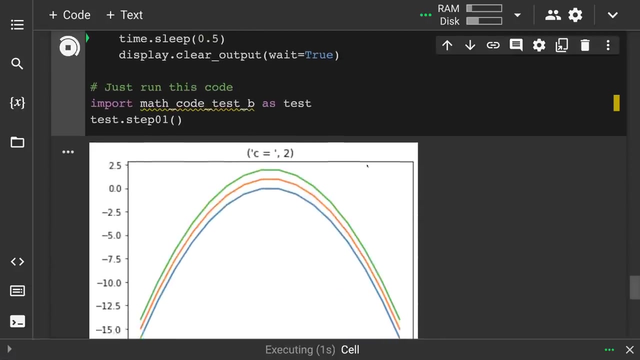 Method. The Argument Is Actually Just In Seconds. Sometimes Sleep Methods Are In Milliseconds, This One Just In Seconds. Play This And Then Clear The 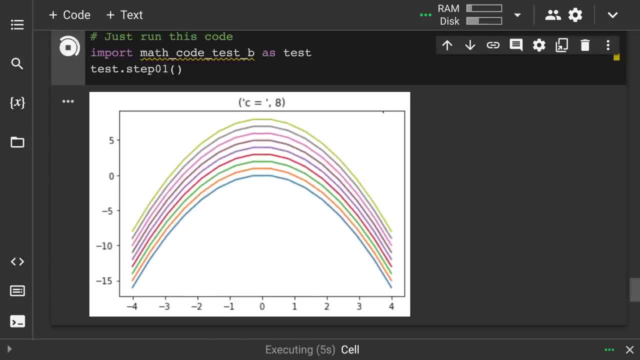 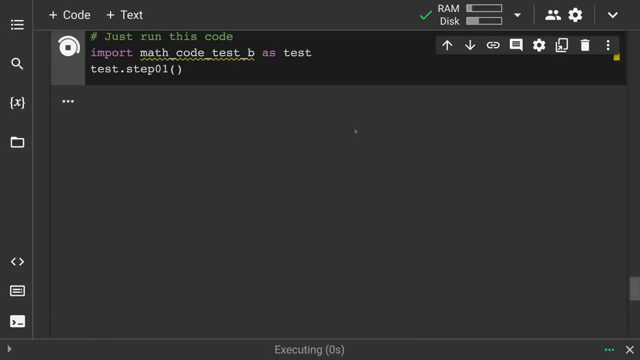 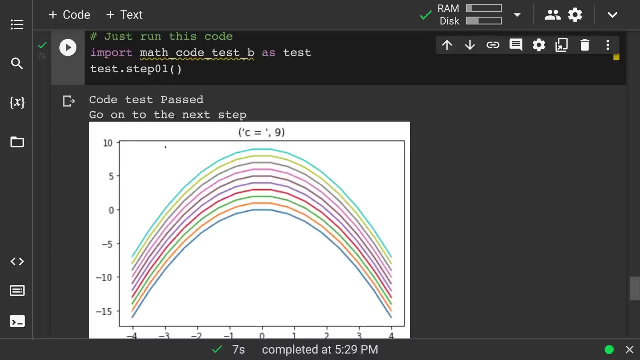 Output, So You See. So All Those Different C Values, We Can See It Grow And We Can Run This Again If You The Y Axis, 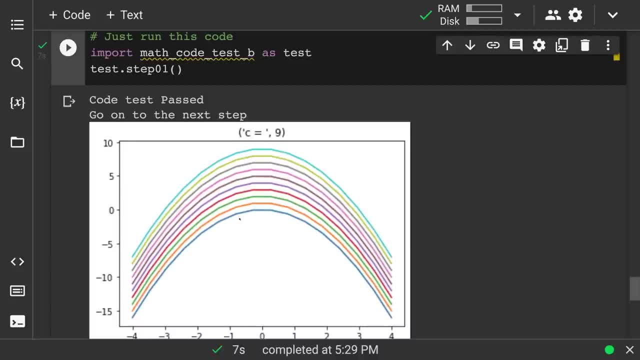 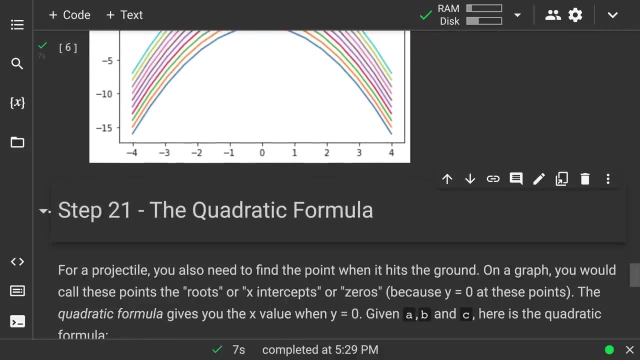 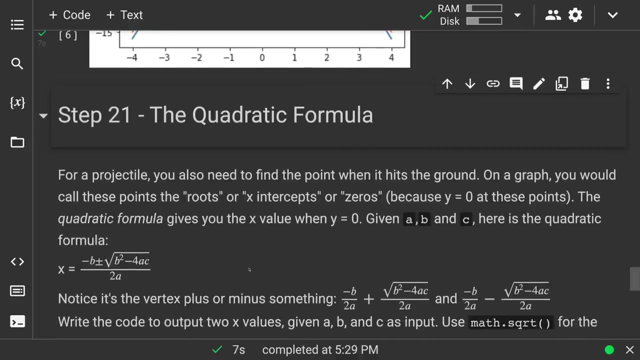 Changed Each Time Because It Accommodated The Larger Graph. So We Can See That Value. All I Have To Do Is You Know Increment C. 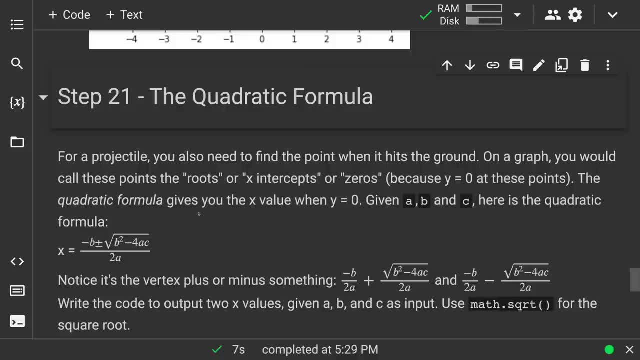 And This Gives You The Roots. Now, If It Was A Projectile, That Would Be When It Hits The Ground. So You Know, That's A. 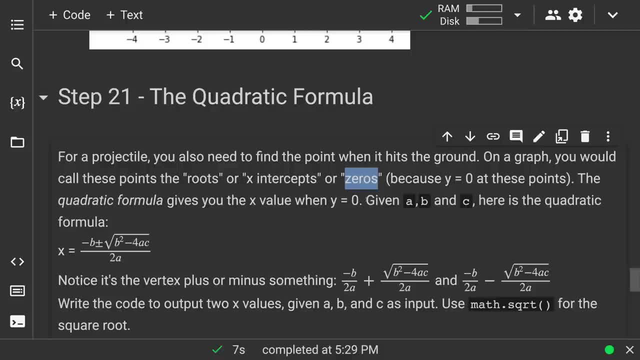 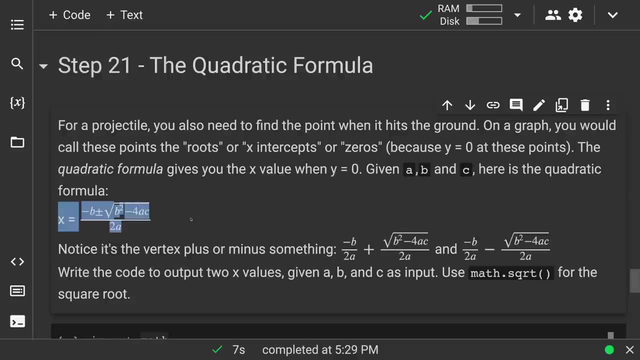 Good Way To Think About Zero. So You'll See It Come Up As All These Different Things. So Now, If I Know A, B And 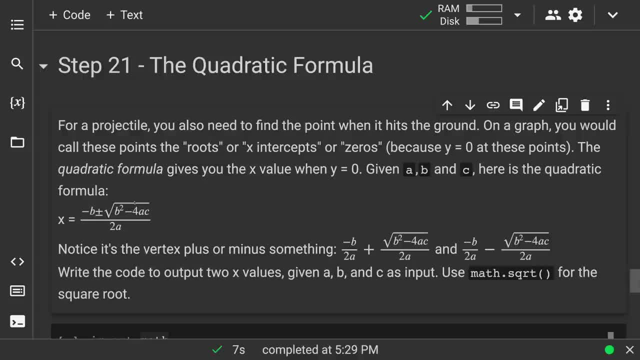 C. Here's The Formula. If I Were To Write It And Notice We Have The Plus Or Minus Because Somewhere Along The Way Deriving 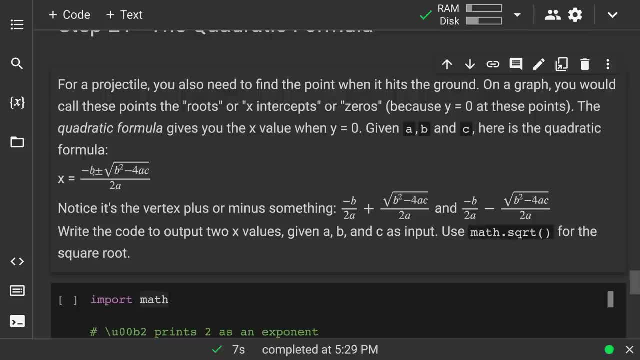 This: You Do A Square Root And In The Square Root You Have Two Possible. This Is The Vertex. You Recognize That Formula Plus This: 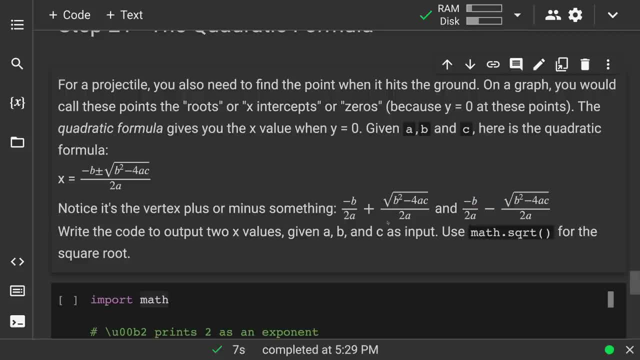 And Then The Vertex Minus This. So You See, That's Another, Just Another Way To Write It, Whether You Have X Value Of The Vertex. 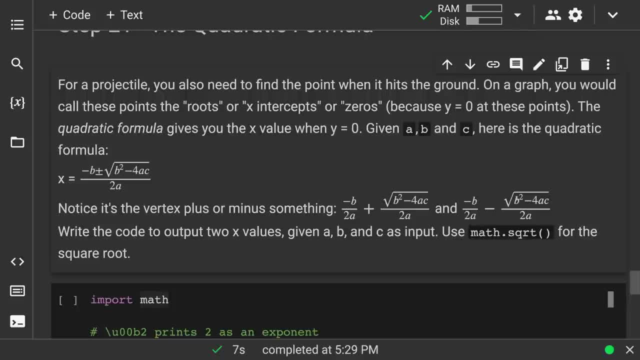 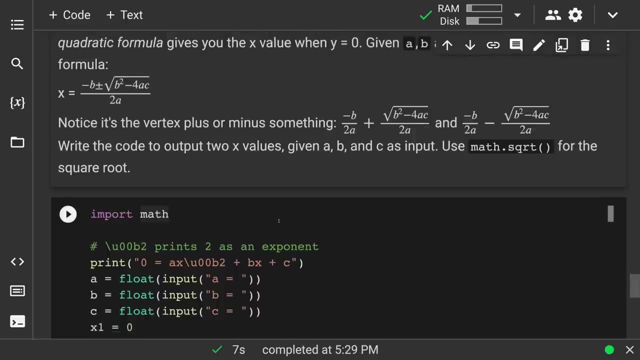 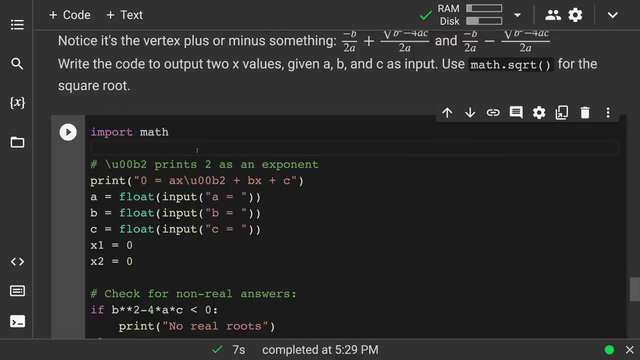 Is Right In The Middle. So It Makes Sense That Value Right In The Middle, And Then Plus Something And Then That Value, That For The 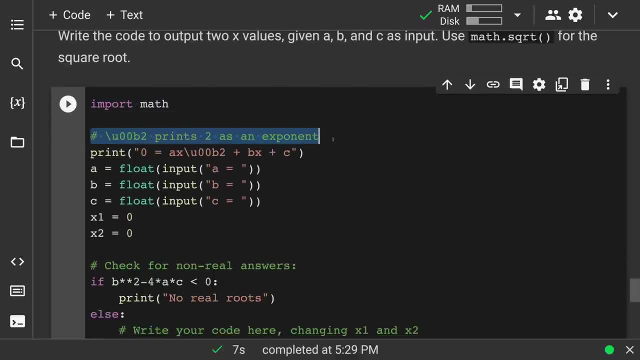 Square Root And I Have It Printed Out Like This, Where I Just Have The Comment To Remind You That That Just Prints To His 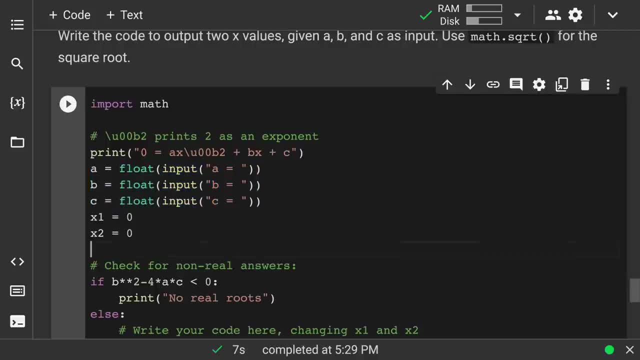 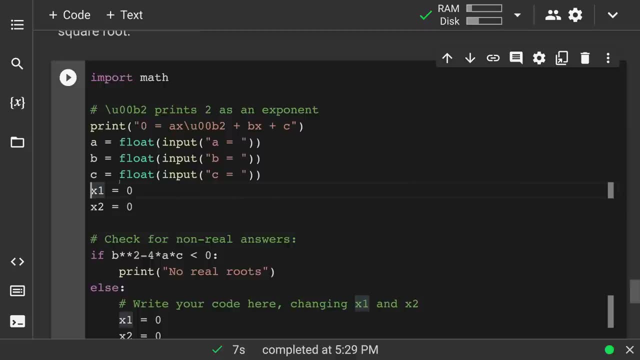 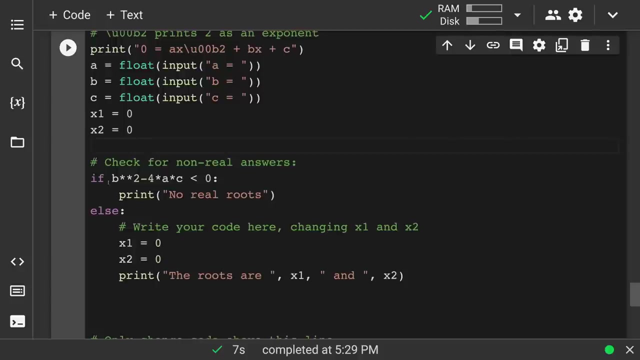 Exponent. So There We Go Now Here. This Is Where You're Going To Check, So I Just Put These Here. Will Define These Variables Here. 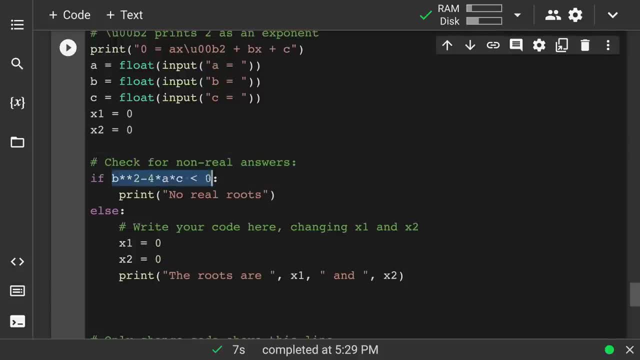 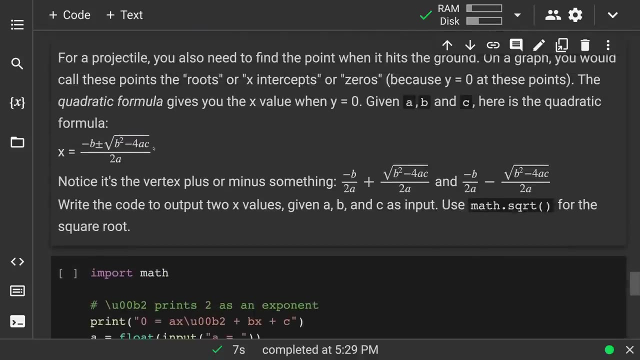 There's Zero, But We're Going. Now Notice What This Is: B Squared Minus Four Times A Times C, Because Remember, That's What's Underneath. 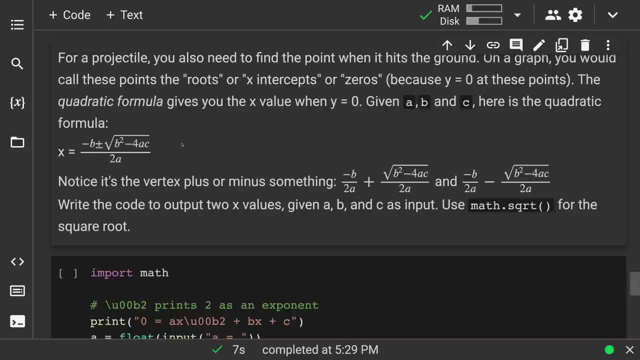 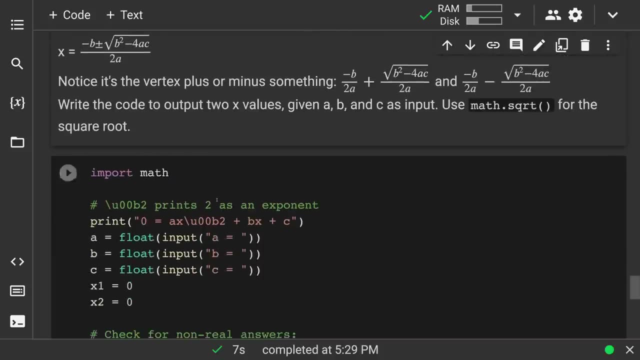 The Square Root Here, And If That Was Negative, Then Your Answer. But For Our Purposes Here We Don't Want A Negative Under The Square. 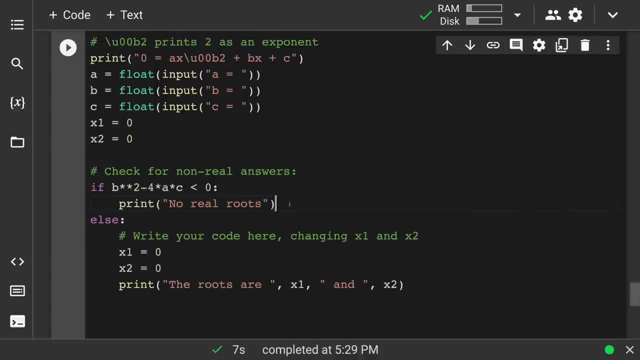 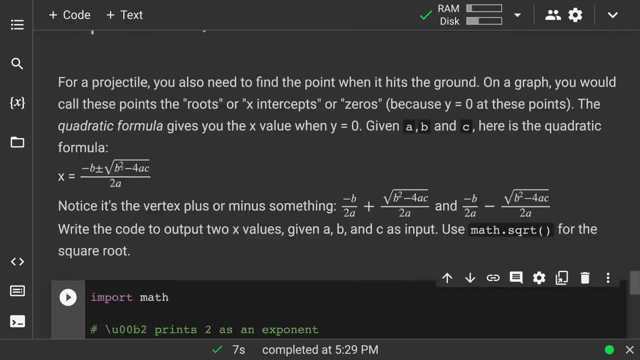 We're Not Going To Imaginary Numbers, So We're Going To Test. If This Is Less Than Zero, Then There's No Real Roots. If That. 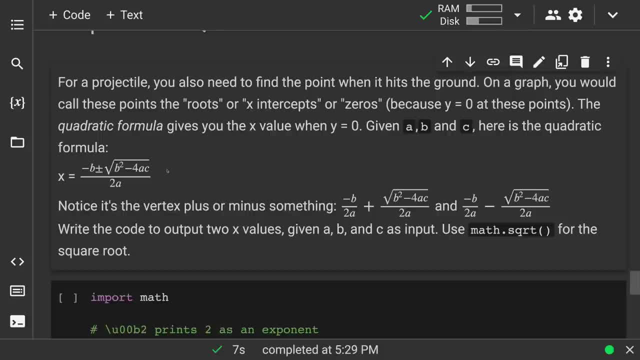 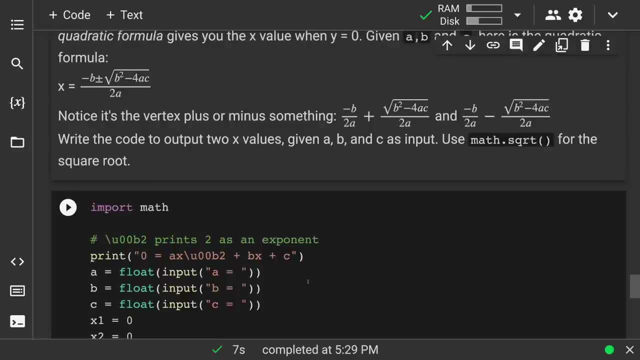 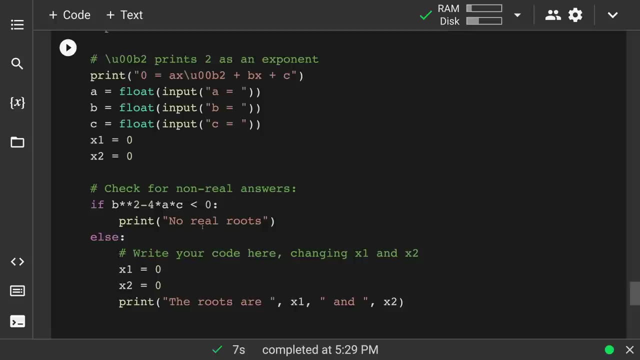 Actually Equals Zero, Then This Plus Or Minus Doesn't Mean Anything, Because Plus Zero, Minus Zero, It's The Same Thing. So If You Touch, 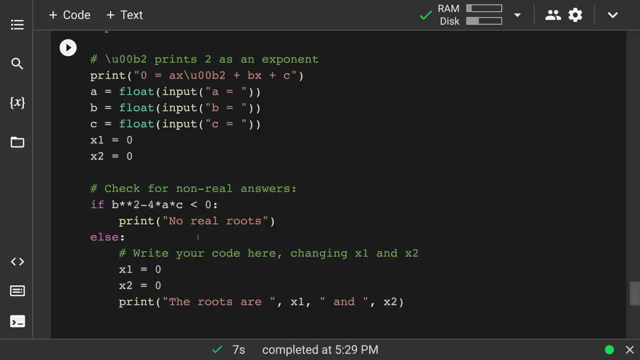 Or Cross The X Axis. So You Could Have That. You Know, Just Parabola, And It Opens Up And Crosses Early, You Know, At 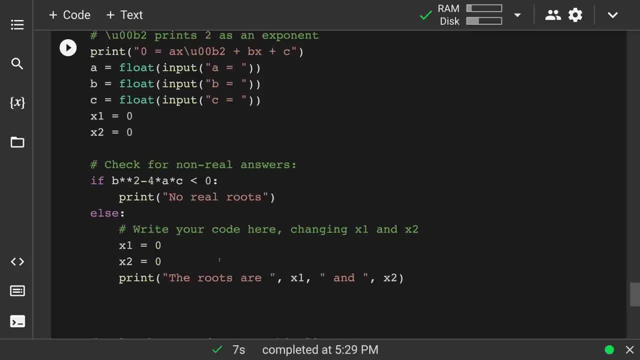 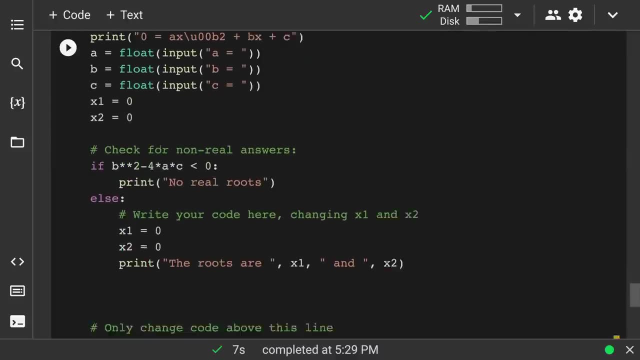 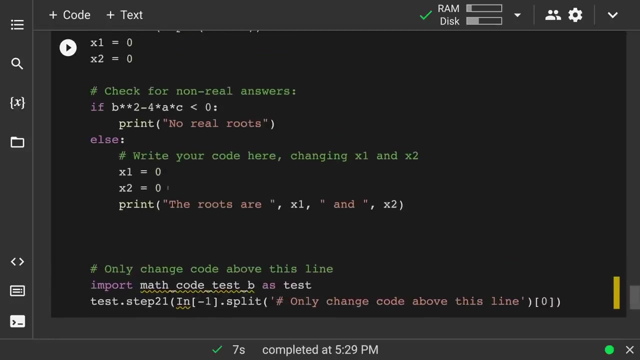 Some Higher Y. So How Are We Going To Translate This, This Quadratic Formula, Into This? Well, We're Going To Do X, One And Two. 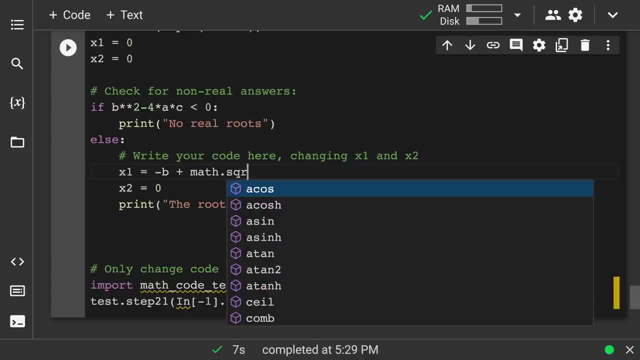 We're Going To The Very Similar Thing, That Is, A Square Minus Four Times A Times C. All Right Now, All Of That Remember Was: 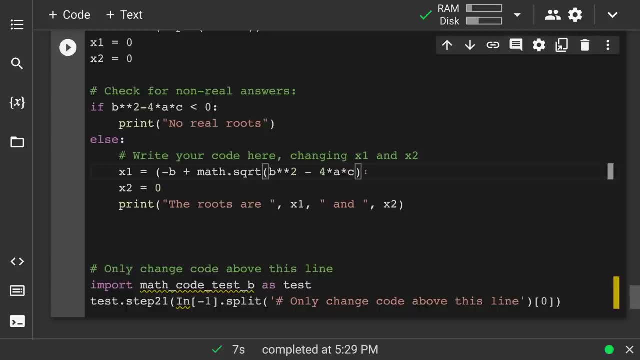 In The Numerator, So I'm Going To Put Parentheses Around. All To Divided By Two. A So Order Of Operations: All This Stuff Python. 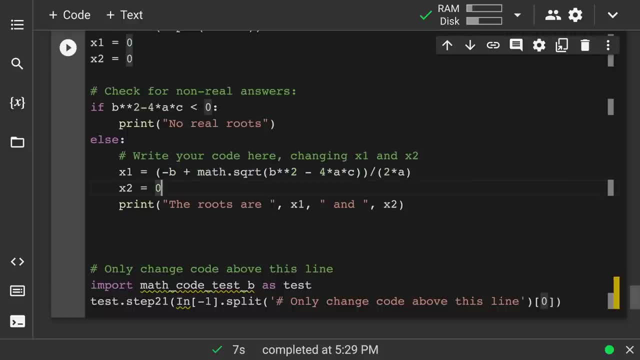 Will Know. But Then Since I Have Numerator And Denominator In Parentheses And Then The Second, So This Is Minus. So All Of Things. 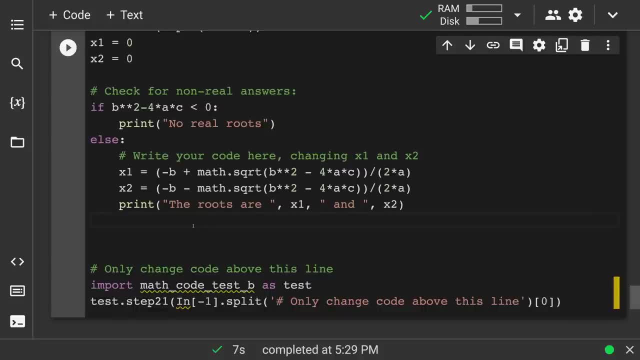 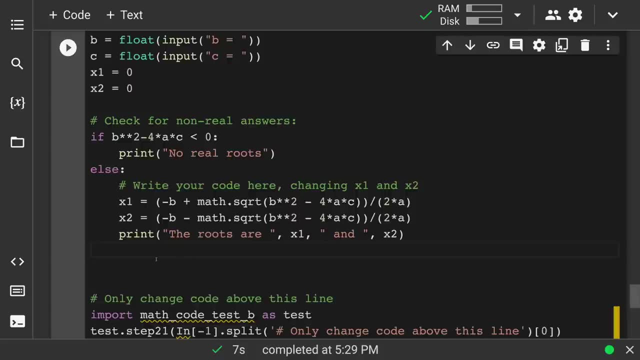 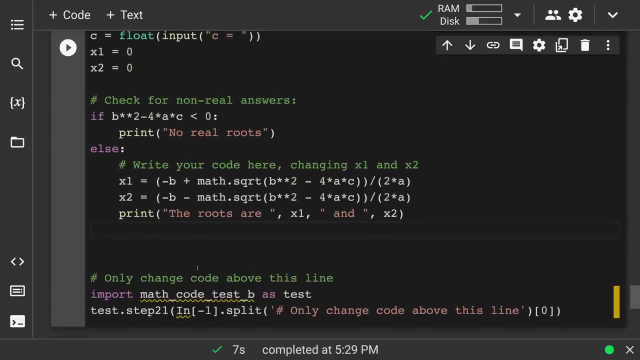 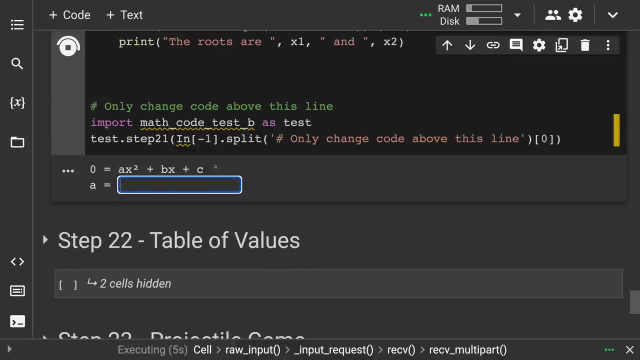 You Can Do So Now. A Lot Of Things You Can Do, You Know, In Solving A Quadratic, Very Often We Do Showing That Display. 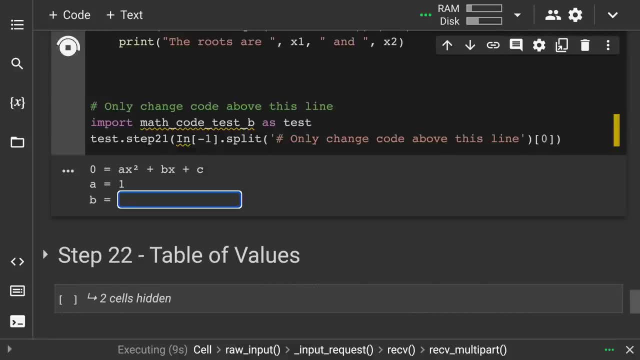 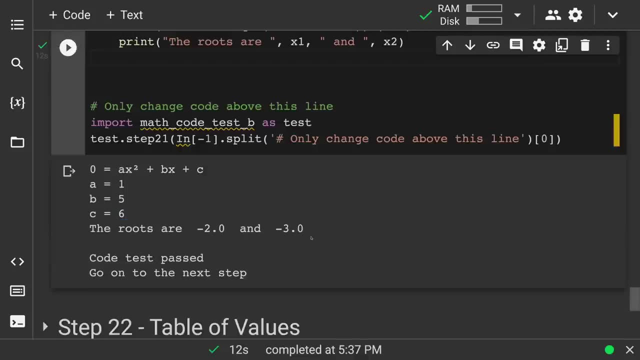 So Let's Just Try Numbers That Work Out Pretty Nicely: One And We Have To Do Five And Six. Let's Try That. Look At. 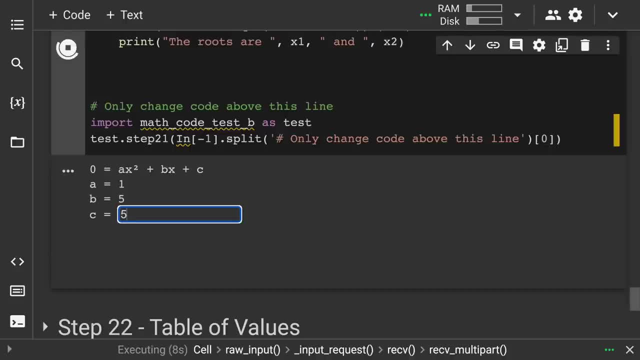 The Roots Five. You See, It Does Have Roots, Definite, Real Roots, But Since It Doesn't, Certain Ones Don't Work Out, And There's Actually 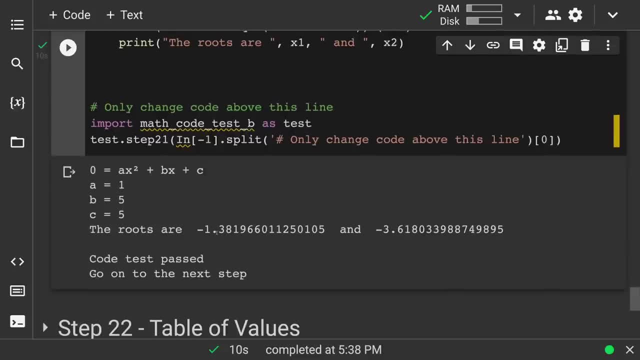 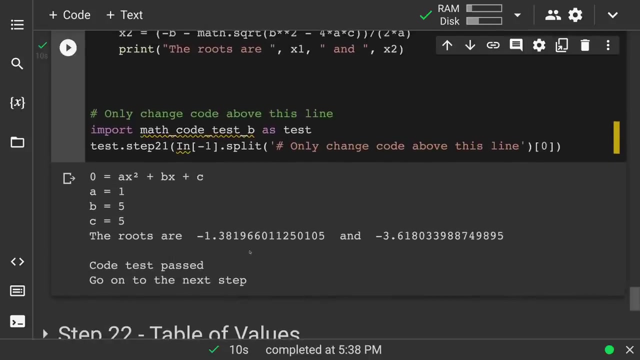 Like A More Complicated. You Know That You Might Have Some Weird Irrational Roots. You Could Round It To. You Know Three Or Four Decimal. 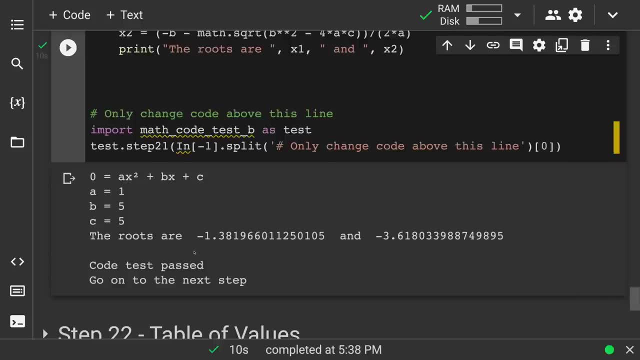 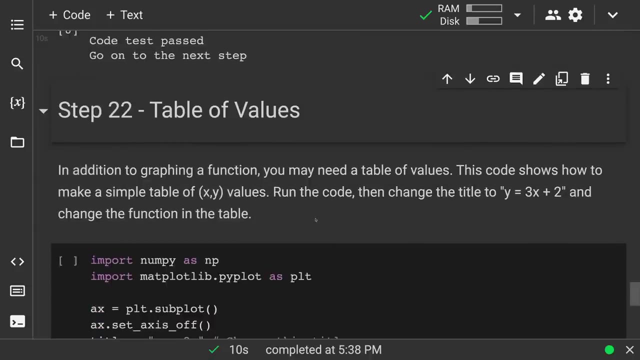 Places, And I'll Leave It Up To You Know, We Can Put These Two Things Together. You Know Some Interesting Things You Can Try, So 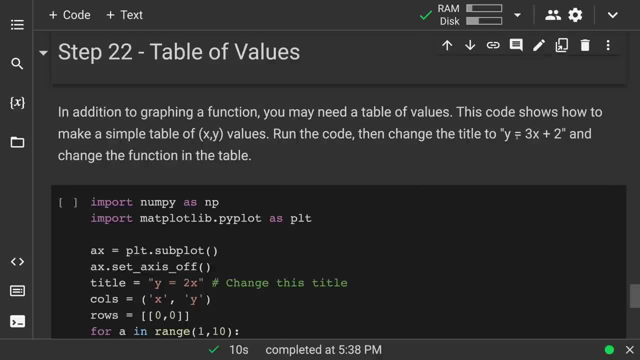 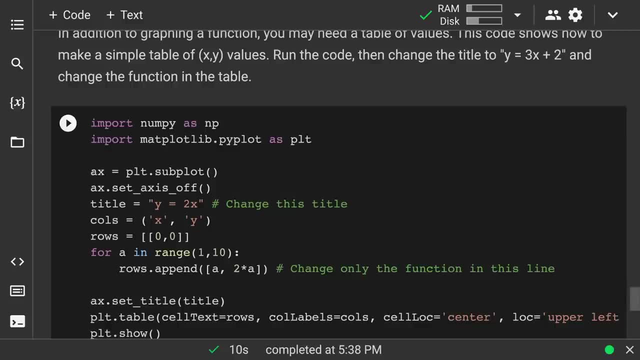 Sometimes The Graph. I Like The Graph But I Know It's A F, I, G Dot Error Comma Axe. I Just Have Axe Equals, So 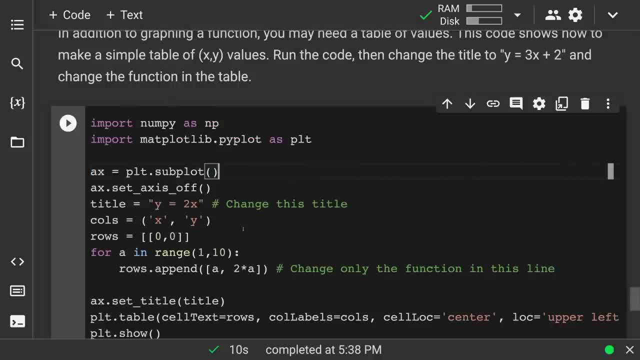 I'm Not Going To Need The Figure, The Graph, I Just Want This Because This Plt, We're Going To Run This And Then Change. 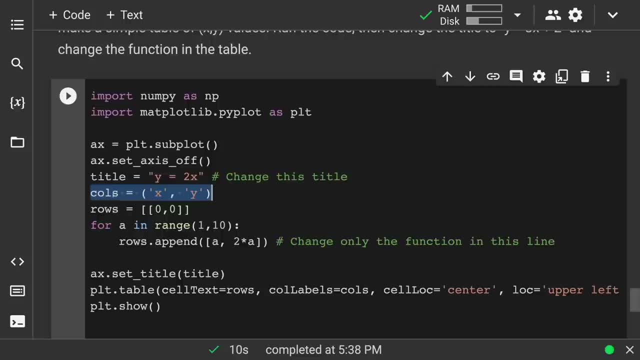 It And Notice How This Works. I Can Define My Columns And I Could Use Another Variable, But I Just Made This Case In The First. 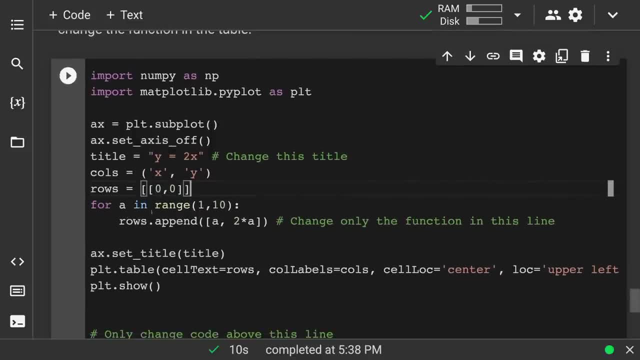 Row X Is Zero And Y Is Zero, And Then What I Can Do Is, In This Case, Since I Have This For A In Whatever, 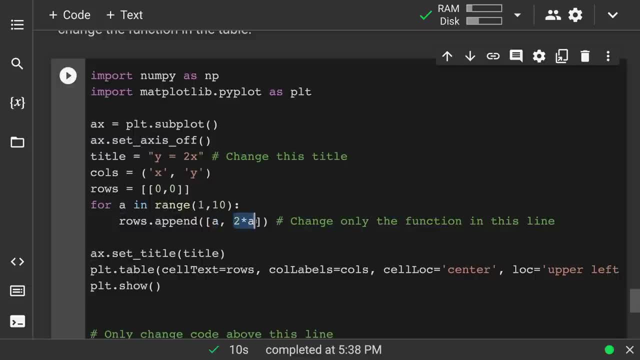 That's Going To End Up Be Well, It's Going To Be One, Then Two, Then Three And Then Two A You Know? Just Something Simple. 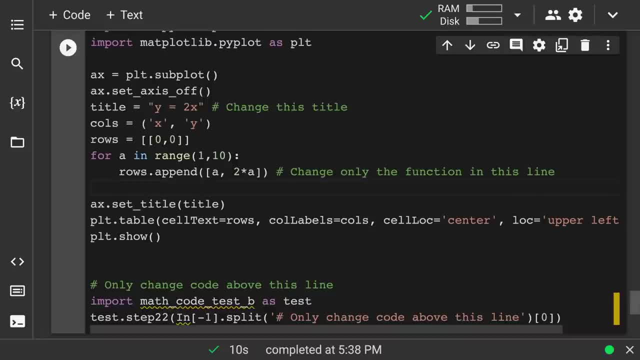 For The Y. So Now, Outside Of That Loop X Set Title. I've Already Defined It Up There, And Then Take A Look At This: 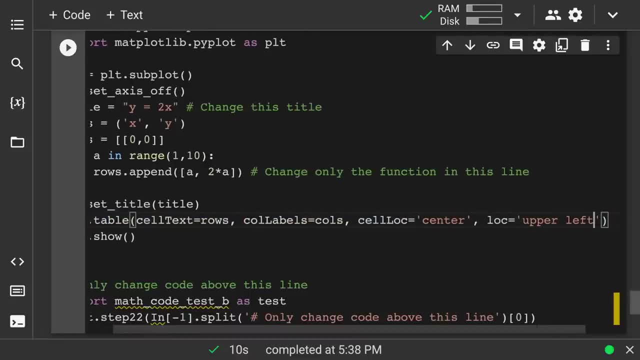 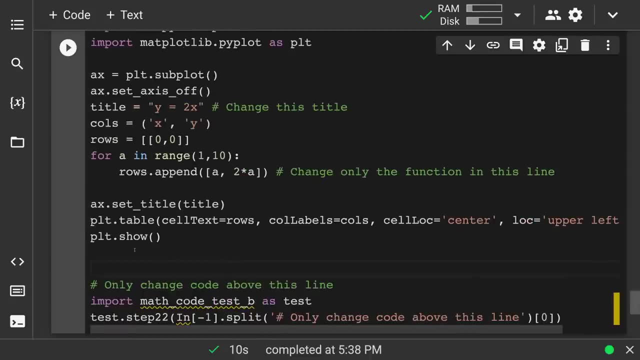 PLT Table And It Takes The Argument To Show You. So It's Still This Last Direction PLT Show, But What We're Showing Is A. 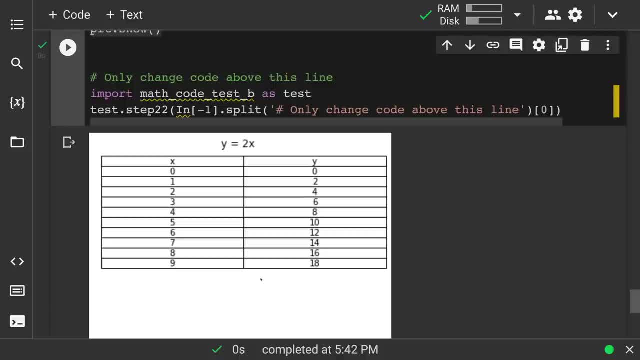 Table Instead Of A Graph, And You See How It Looks. Now You And It, As This Is Leading To Data Science. This Is Like An 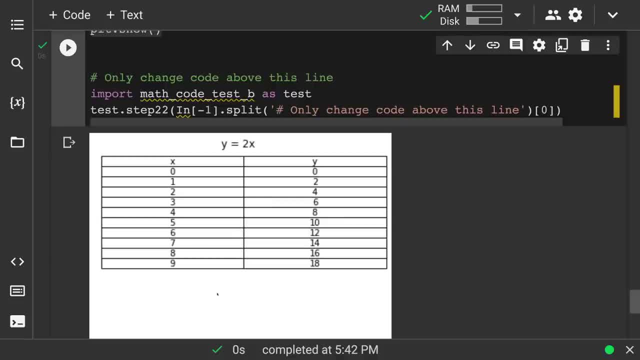 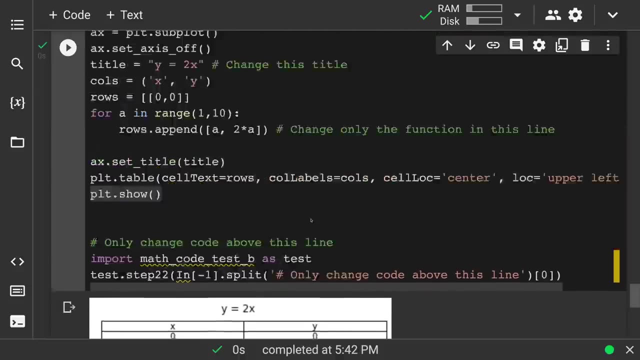 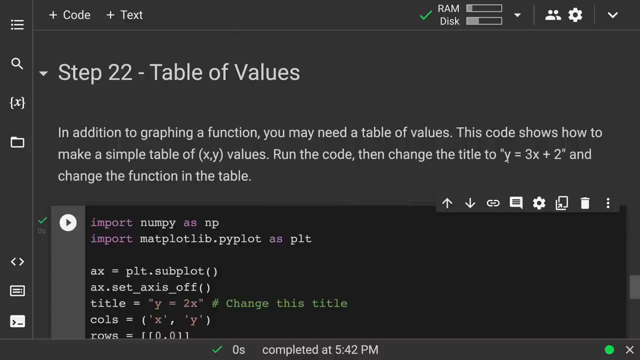 Introduction. There's Some Things You Can Do To Generate A Table, Values Or Things Like That, And You Could Always Make This Quadratic Or Whatever. 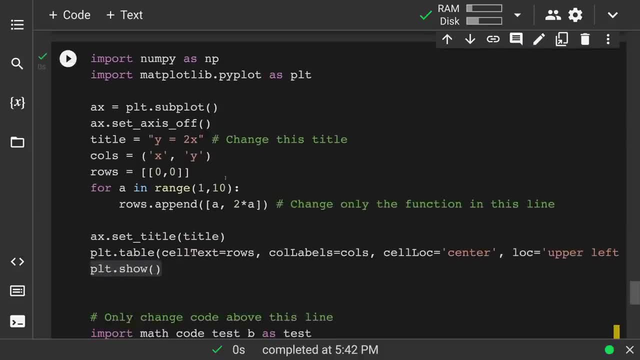 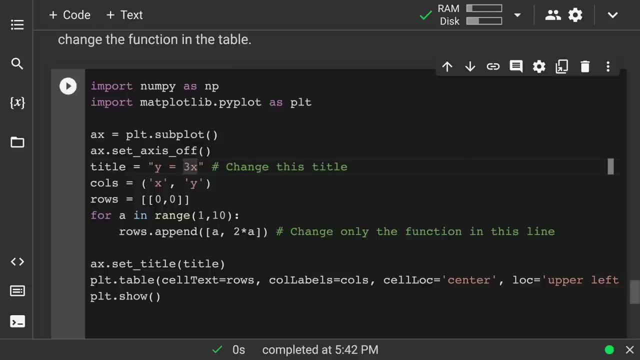 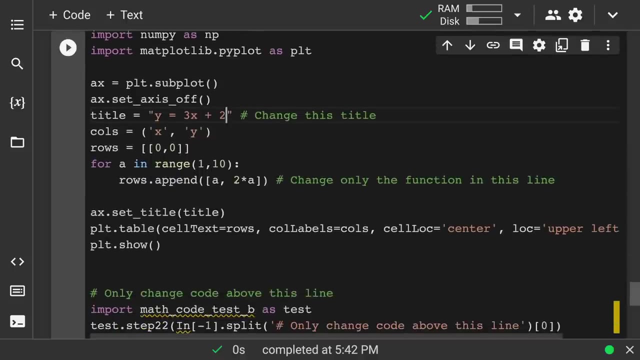 You'd Like It To Be Again, Just For Simplicity, To Illustrate The Table Itself. I Wanted To Keep It. This Is Where I'm. 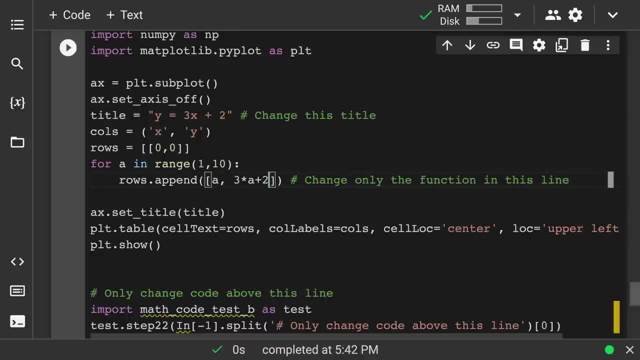 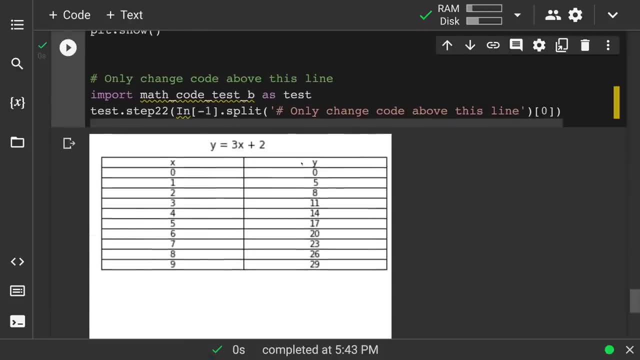 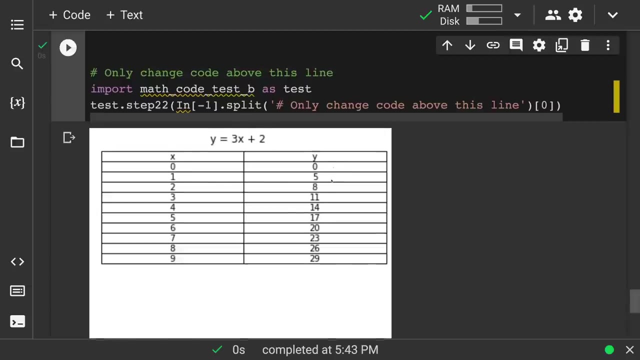 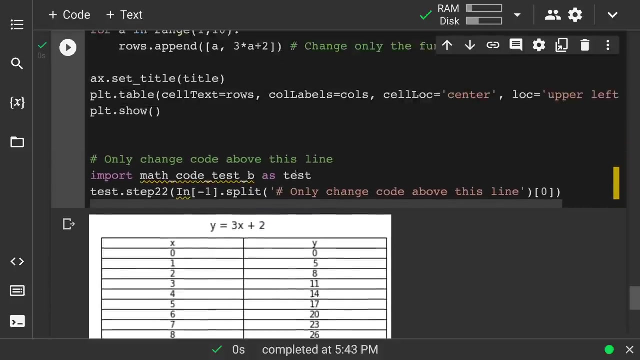 Going To Take It, And A Is My X Value, So It Would Be Three Times A Plus Two. There We Go And We Run It. 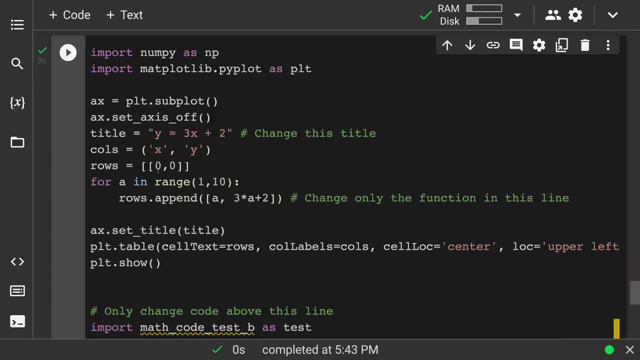 To Now. One Of The Things You Can Do Is You Could Keep This And Then Start The Range At Zero And Remember For The Range. 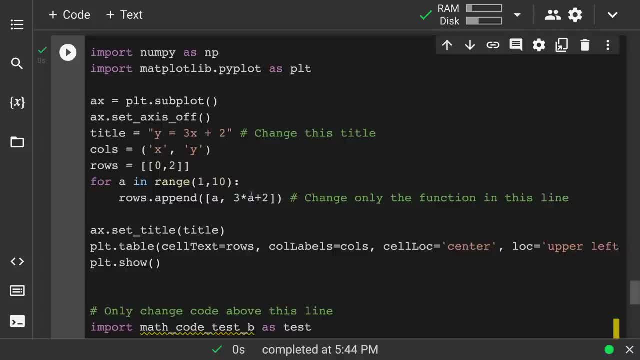 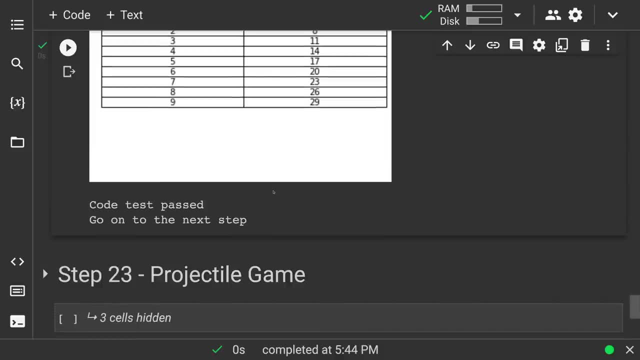 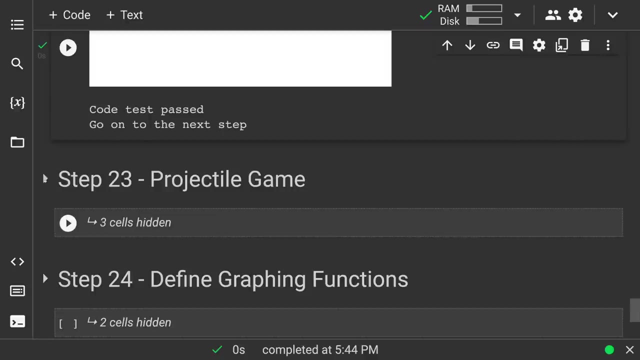 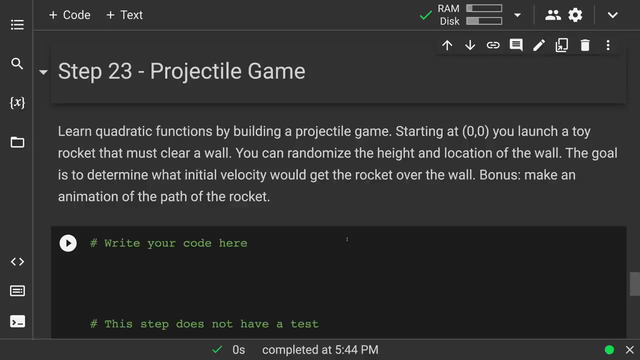 At Zero. You Can Be One Time. So There We Go. We Have Our Table, Okay, So Different Ways To Display, And I Just Wanted To 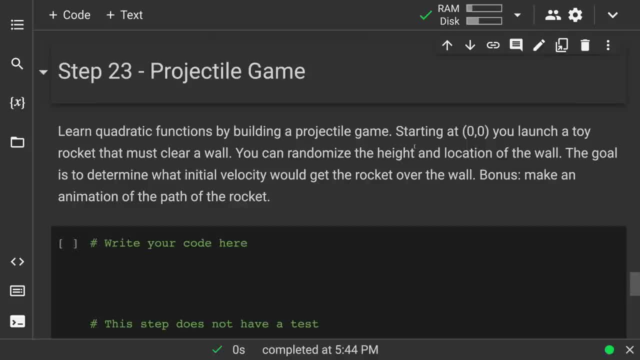 You Know, Have A Nice Interesting Mini Ball Game. So What This Would Be Is Remember Knowing Where You Are Starting From. You Could Randomize. 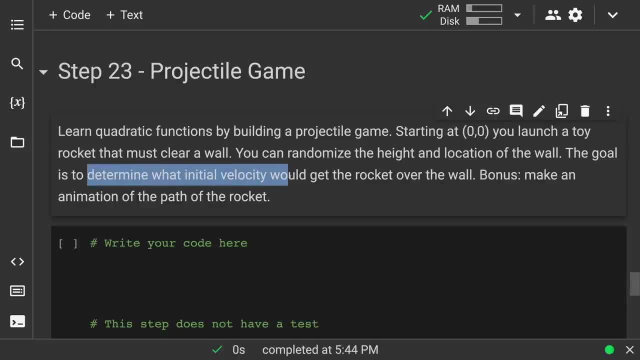 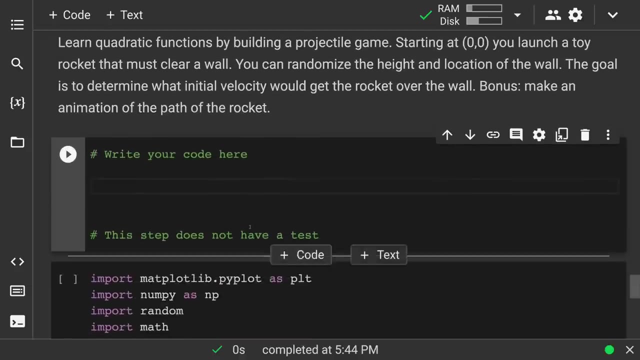 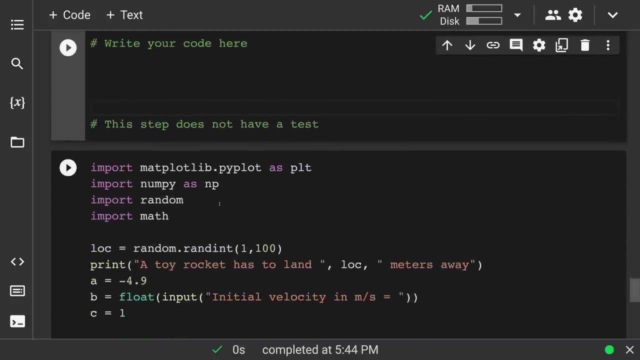 The Height And Location Of A Wall And You Have A Animation Path Or You Could. You Know There's Some Other Things You Could Do. 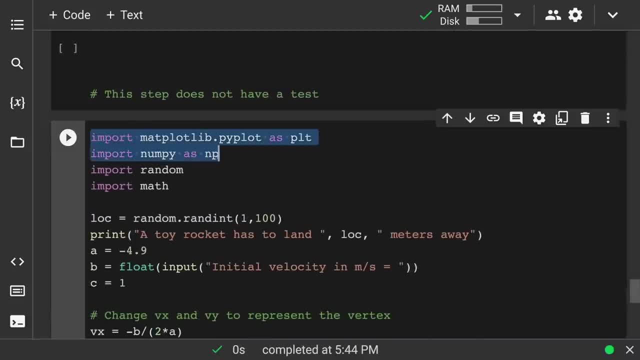 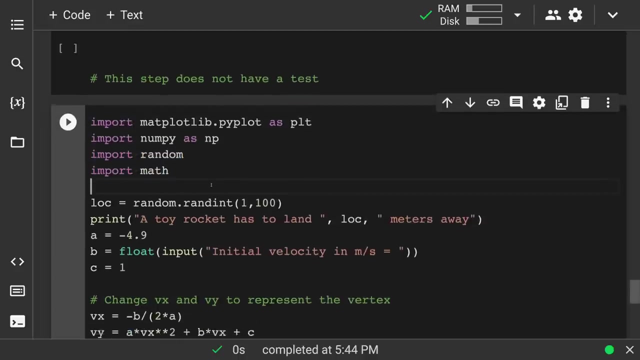 So I Left This Here For You To Write, But I'm Going To Show You A Lot Of Things From There, And I'm Also Going 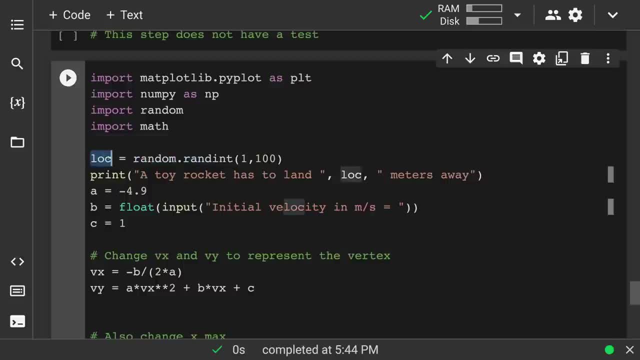 To Import Random And Import Math. So Here I. Just Now I Made This A Modification, So This Is The Location Of, Like A Finish Line. 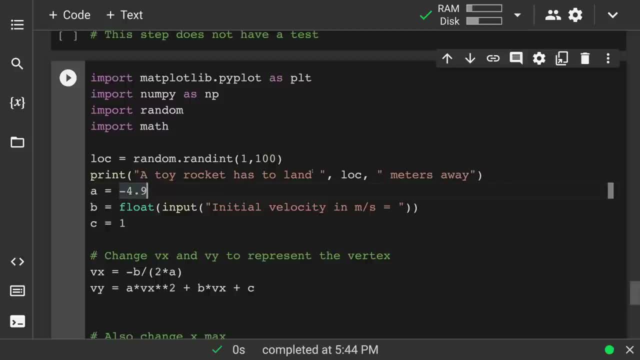 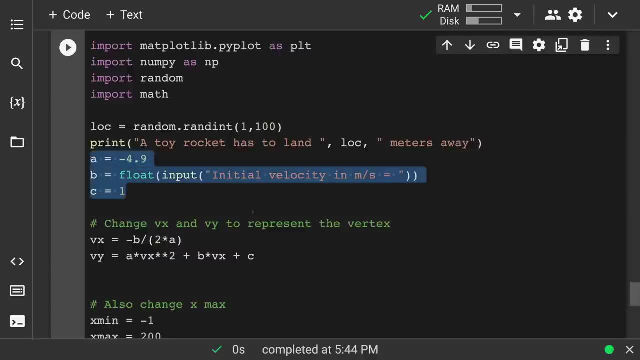 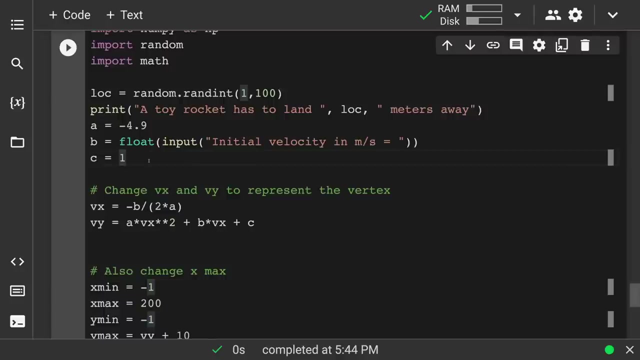 So Here's This Random Integer Between One And A Hundred, And Then It's Going To Print That A Toy Rocket Has To One It You. 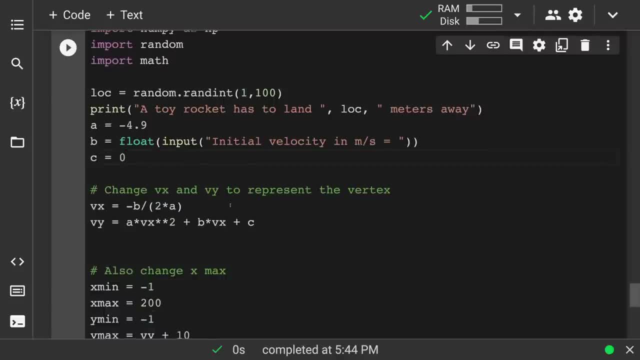 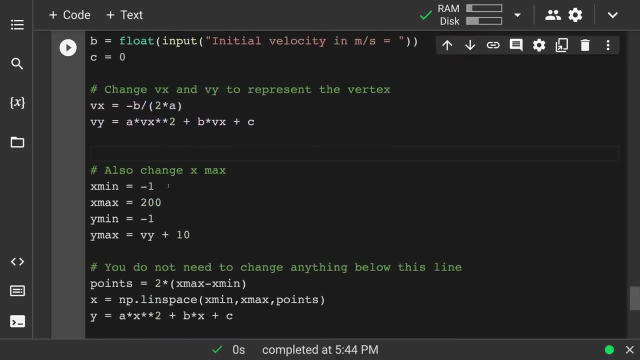 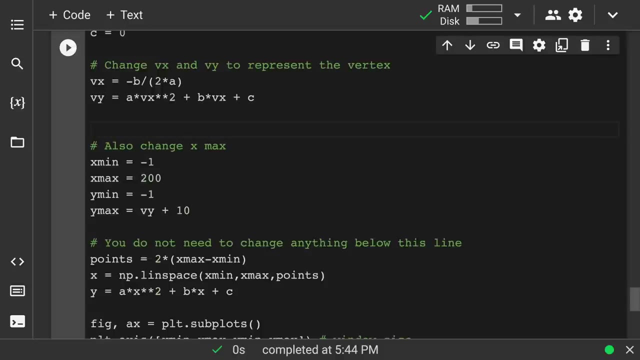 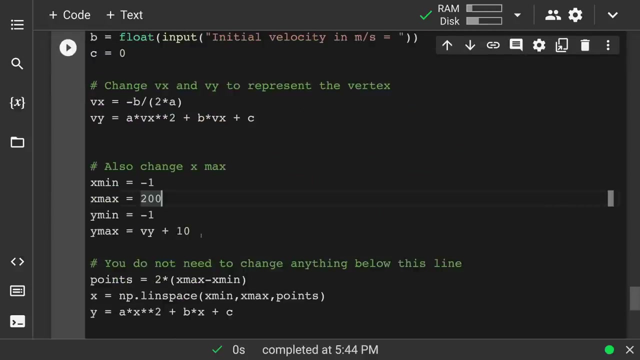 Know Just Because, But It Really Could Be Zero. And Then Same Things. We Want To Represent The Vertex Here And The X? Min What I 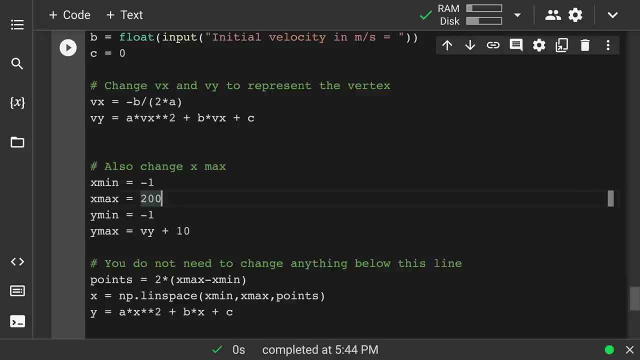 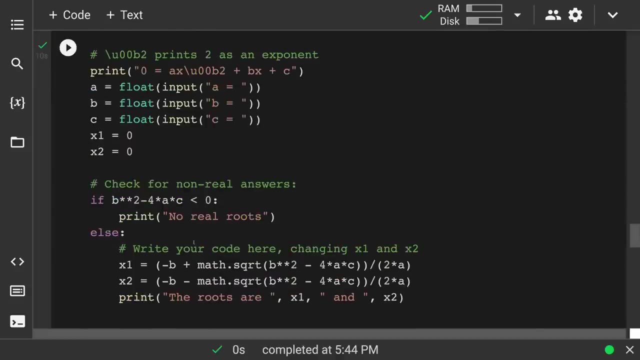 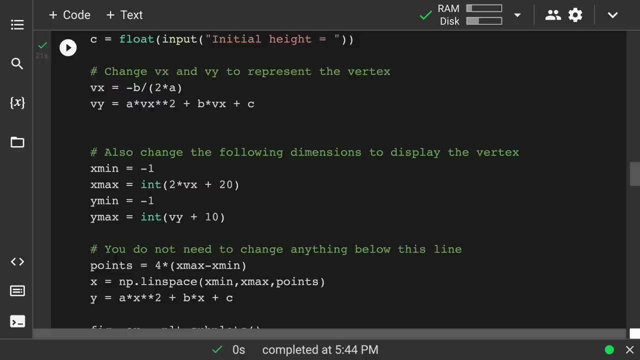 Would Do So- And The Y Maximum. I Left It So That You Could See Where The Projectile Goes, But We Could Always Go Back To 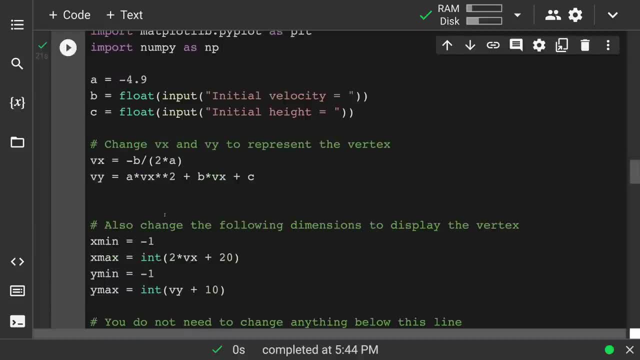 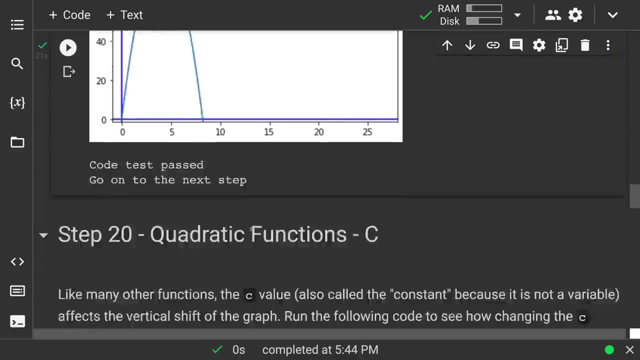 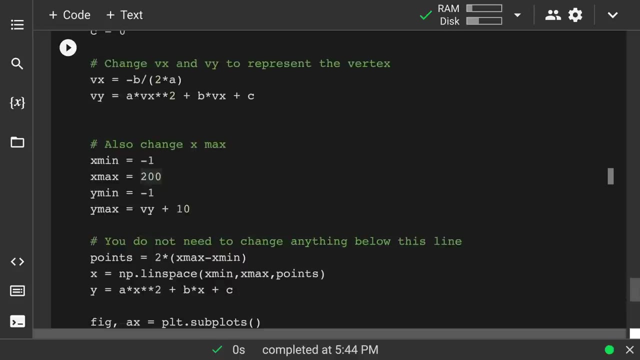 What We Were Doing Before: X Min, X Max. We Could Always Copy These, Because That's What We Want To Do Here. We Want To 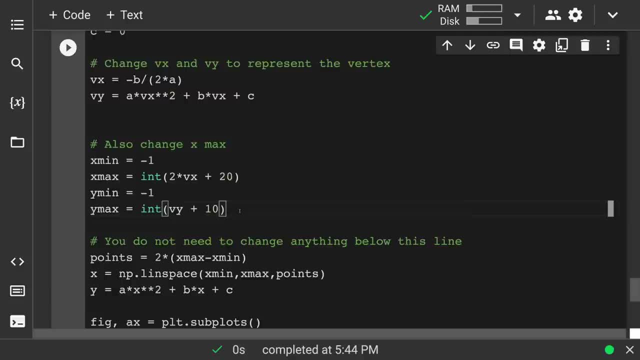 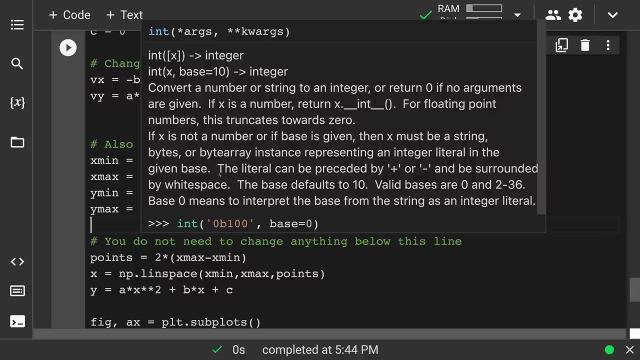 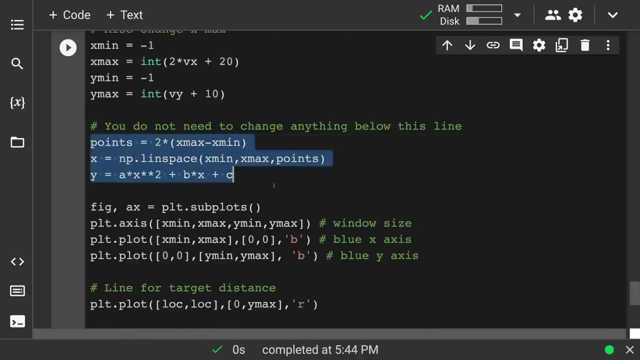 Put These In, And That Was That Was The Way We Could Have. Now. This Would Be Fine, Because Wherever That Wall Ends Up Being, 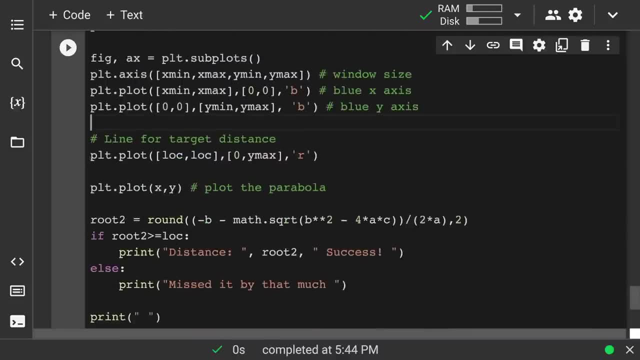 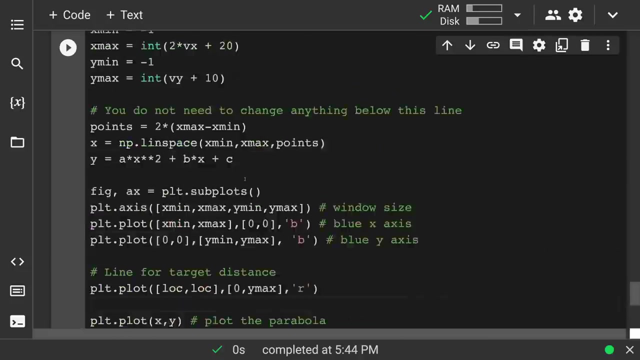 Or The Finish Line. This Is Still Going. It Will Still Print Everything All The Way Up To The Top. Here, Location, My Two X Values: 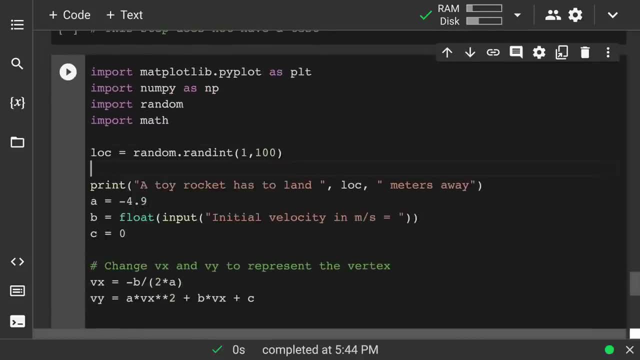 And Then From Zero Up To Y Maximum. So That's Just Going To Be A Line. Where Do I Want This To Be? I Want 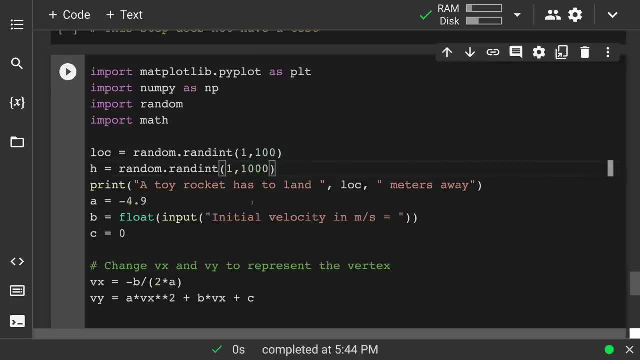 This To Be. I Don't Want Hundreds, Probably Plenty. You Could Even Make It A Thousand. Be Surprised, You Know These Are So If 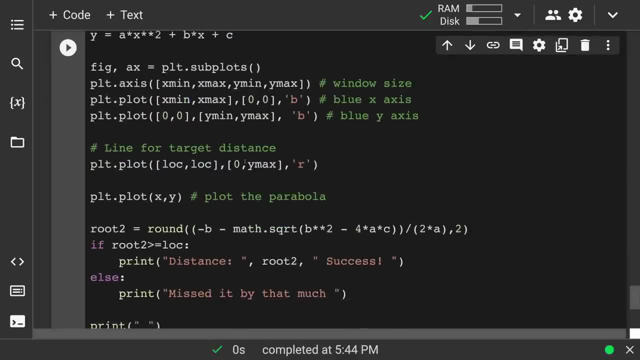 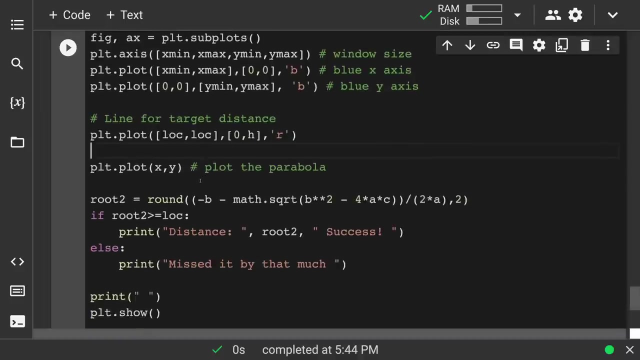 H Would Be. The Height Of The Wall Would Just Be H. So That's The Slight Thing In Looking At This Lot Of Times, The 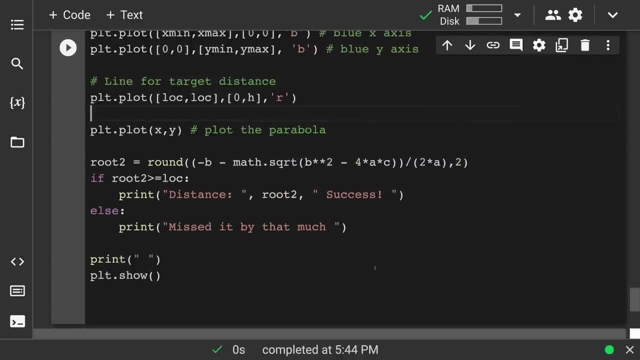 Wall Lot The Parabola. Now, Notice, I Have The Roots And I Picked Just One Of Them And, As It Turns Out, Because Of 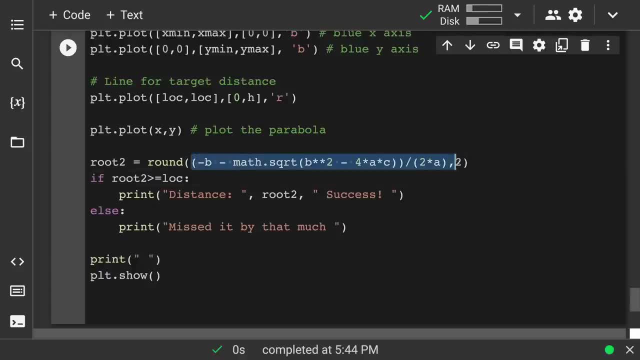 The Way You Know A Is And The Way It Displayed. I Wanted Around This One, So Round To Two Decimal Places. So Here We. 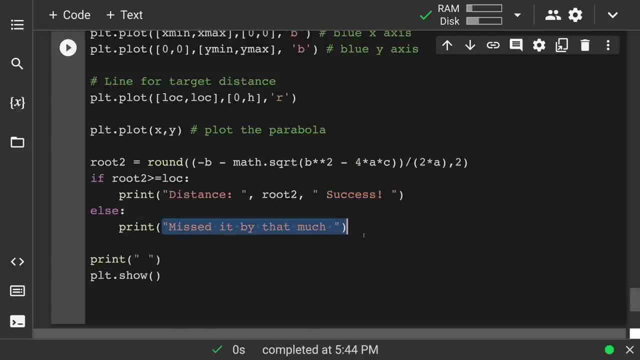 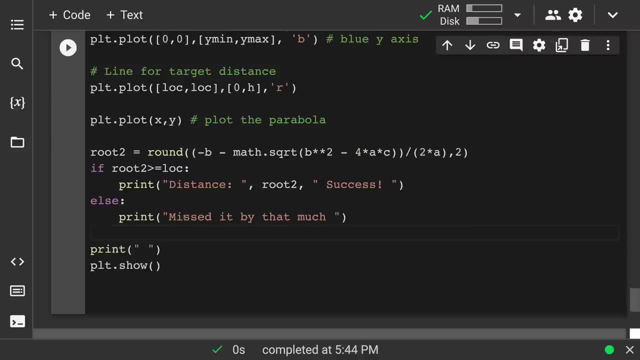 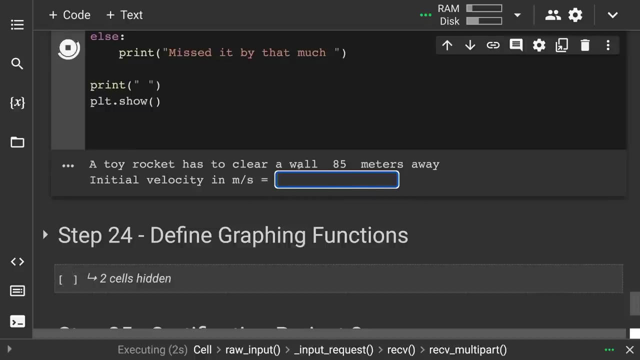 Have If Root To Is Greater Than Or Equal To, This Is It? There Is Actually No Test For This, But You Could See So Here. 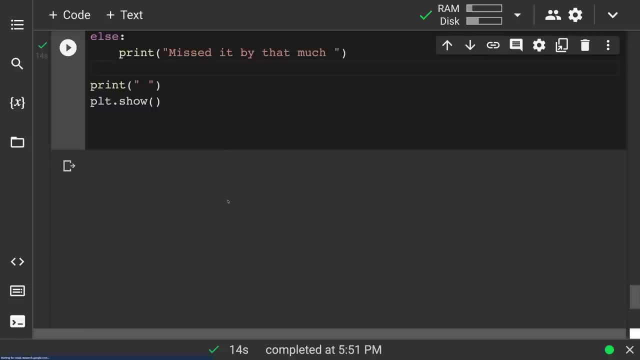 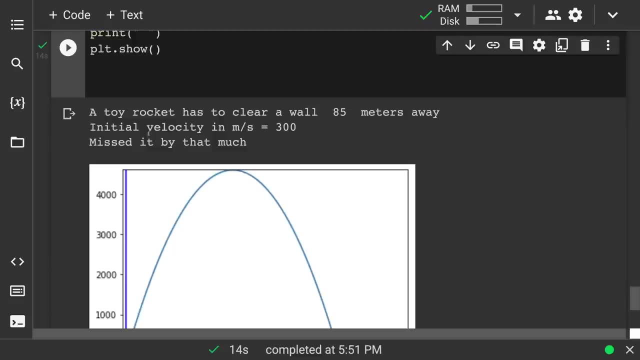 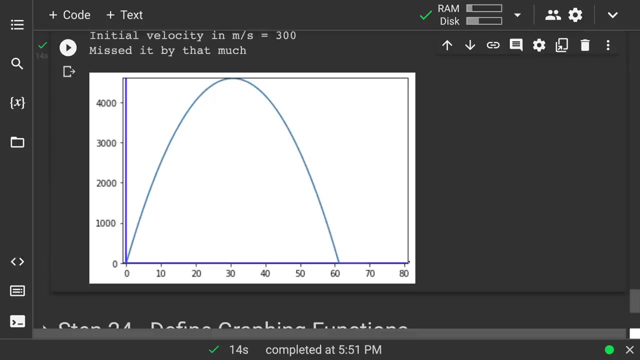 We Go. A Rocket Has To Clear A Wall 85. Meters Away Initial, And You See, Then We're Still. We Didn't Clear, So Missed. 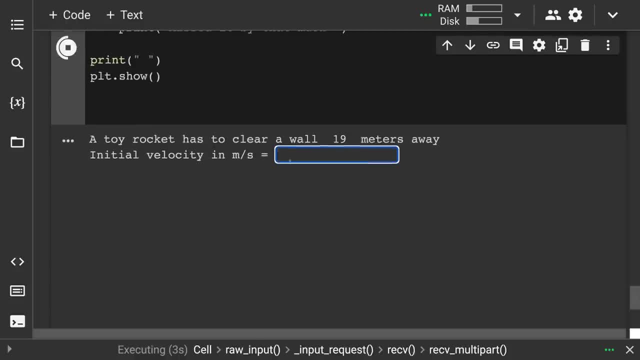 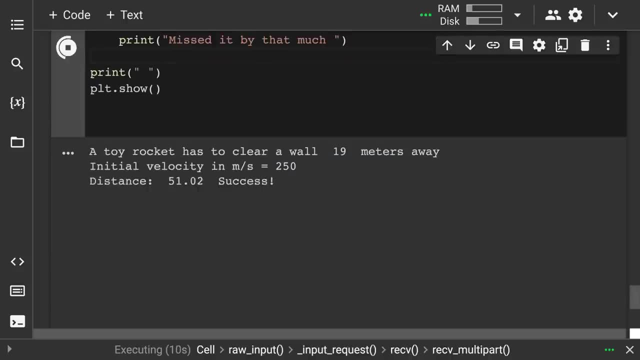 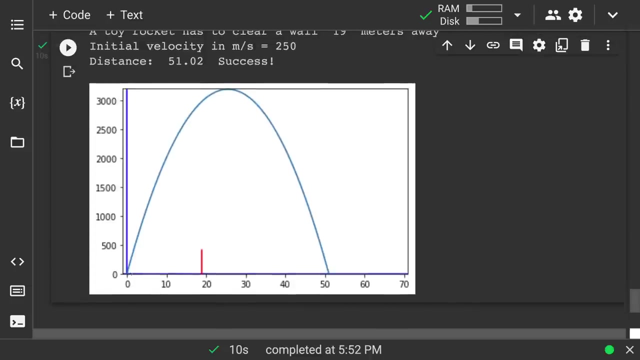 It By That Much And You Can Run It Again Now Other Things You Can Do With This. So Yes, We Did Clear. Now Some Of 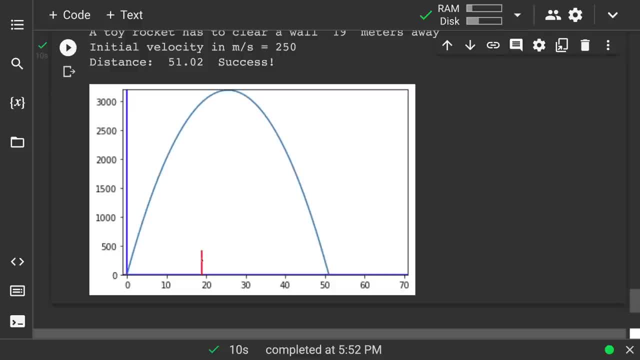 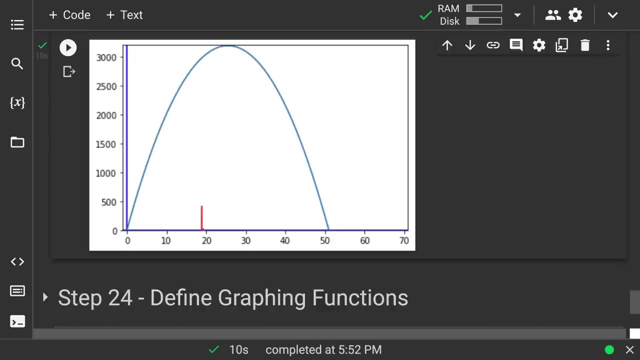 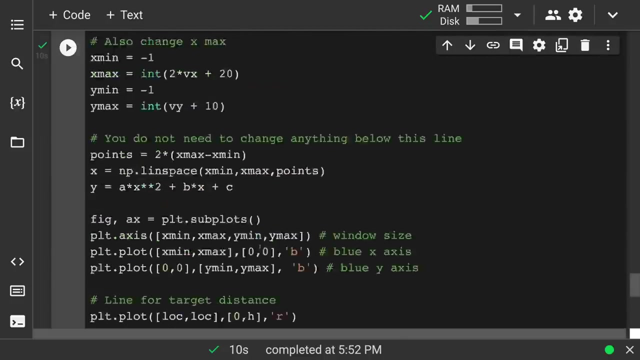 The Other Things You Can Do Is You Could Take This Even Further And, Knowing That Distance, Take That As Your X Or You Could Modify. 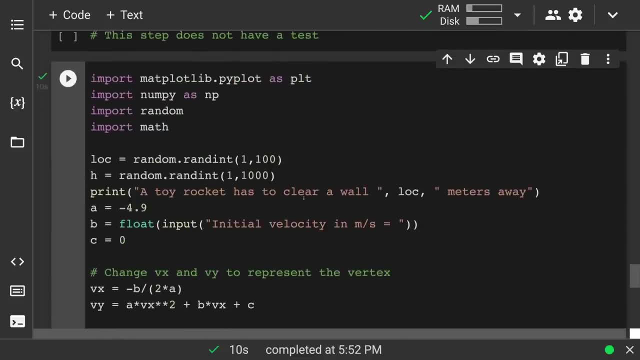 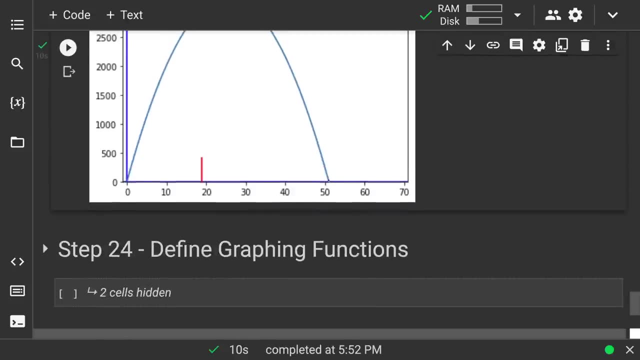 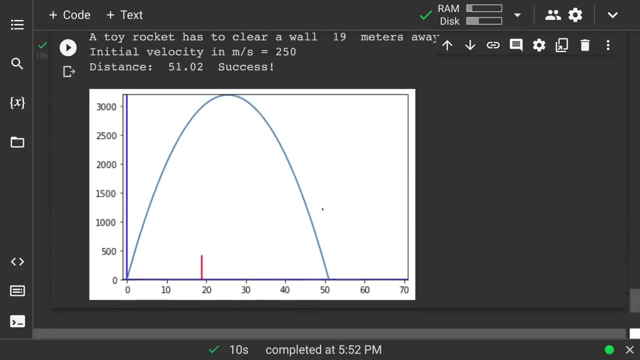 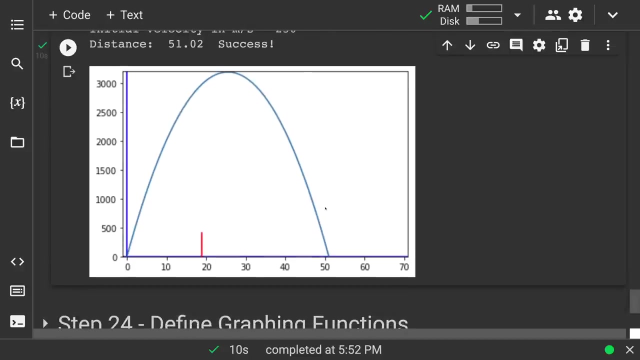 This Game To Say That It Has To Actually Get To A Certain Distance, Not Necessarily That Distance Or More, But Maybe You Say All. 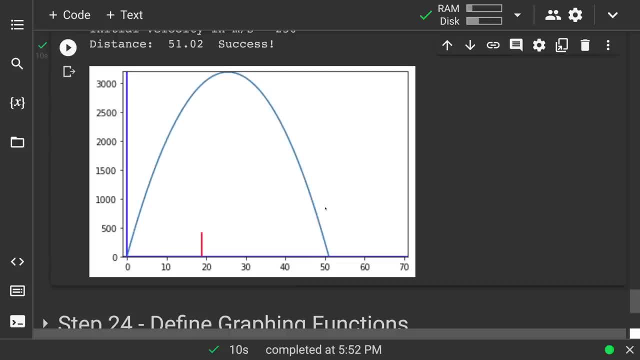 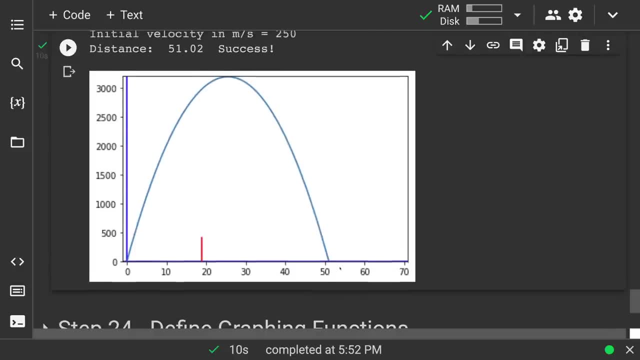 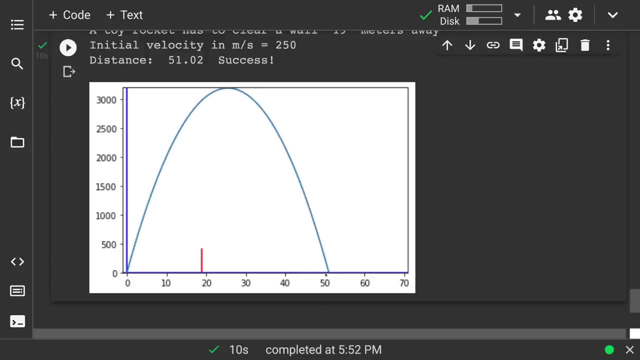 You Could Write The Code To Calculate The Projectile That Will Land Exactly At That Spot. So There We Go Now For This. You Upward. 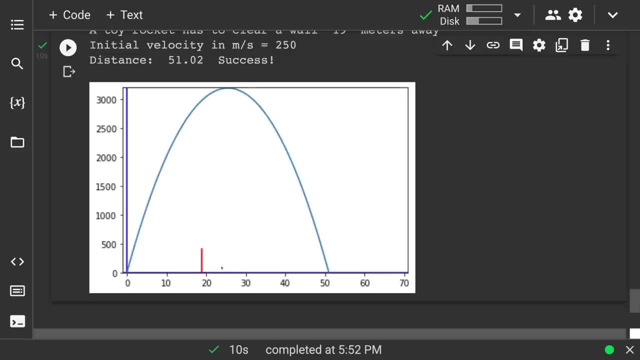 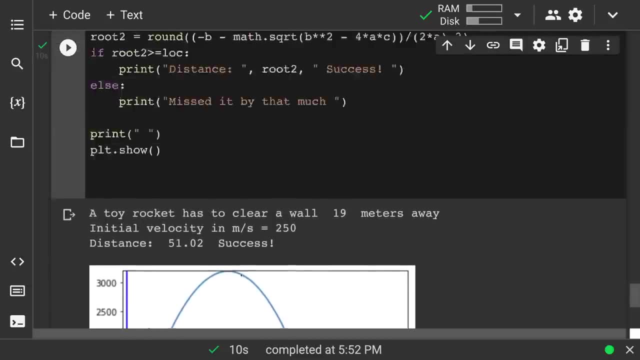 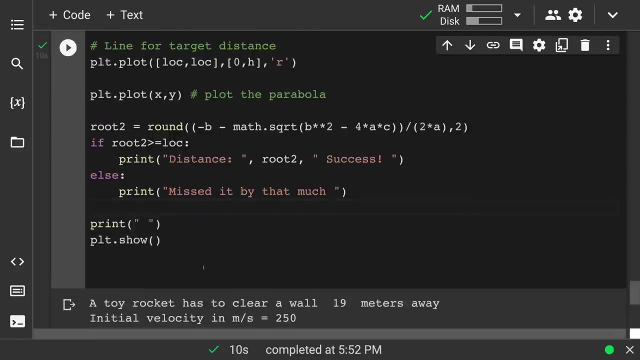 Motion One Of The Ways, And You Can Use That To Calculate Some Formulas And, As I Said, We'll Get Even Better Formulas As 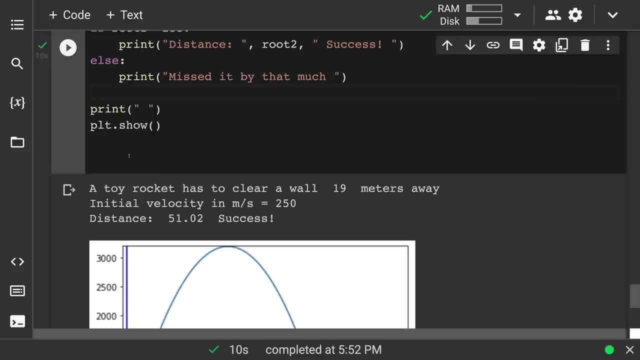 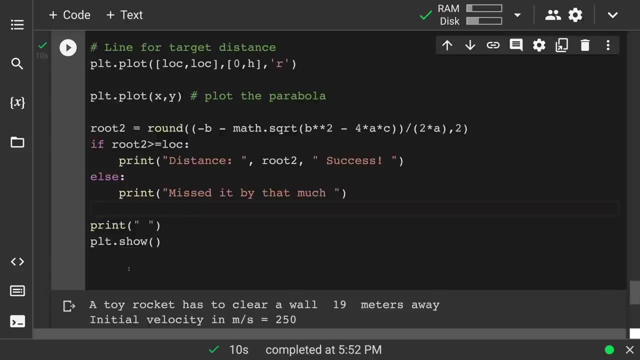 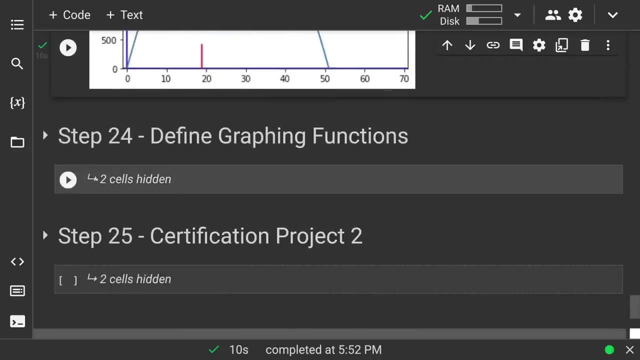 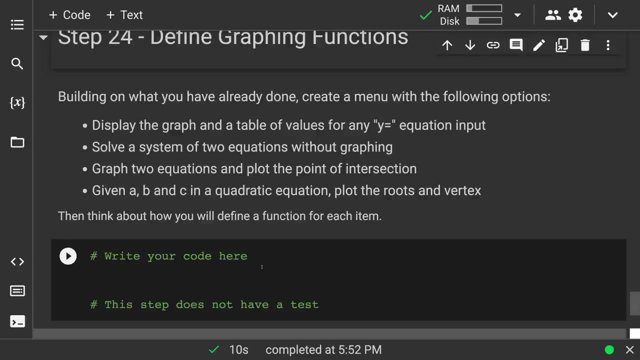 We Get Into Pre-Calc Because We Will Do Things To This And You Have To How Many Ones You Get Correct. But There You Go. 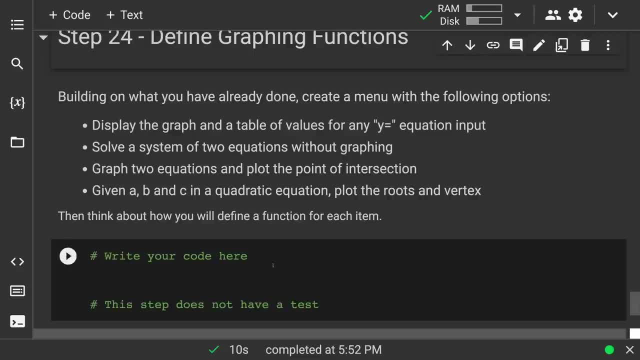 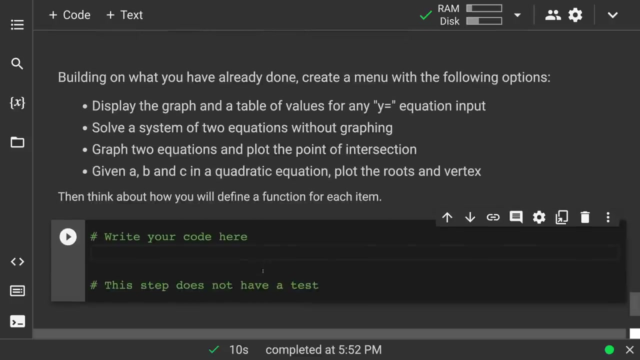 The Projectile Game. Now Continuing On This, This Is Going To Be More Like Working Through Everything Else In This Course. You Might Have Some Of. 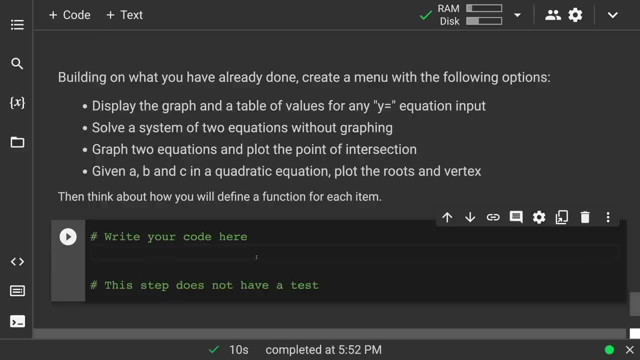 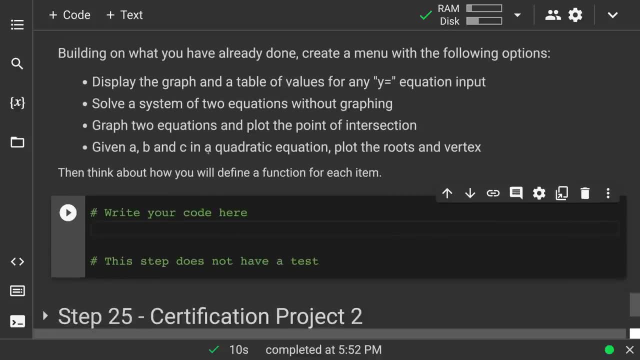 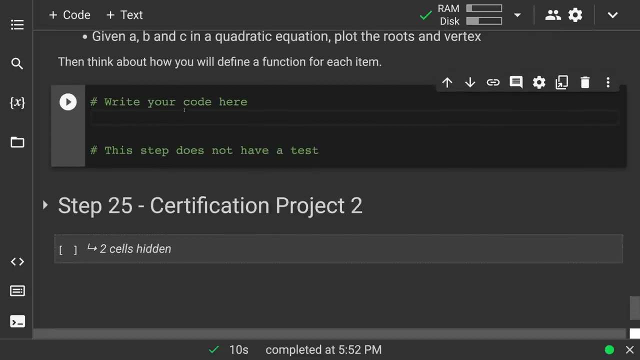 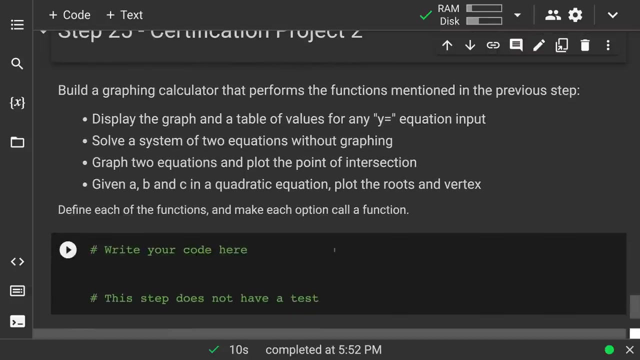 This Already Put Together, And That's Where This, The Certification Project Here, Is. You Know How You Get Functions, Because Then You Get To The 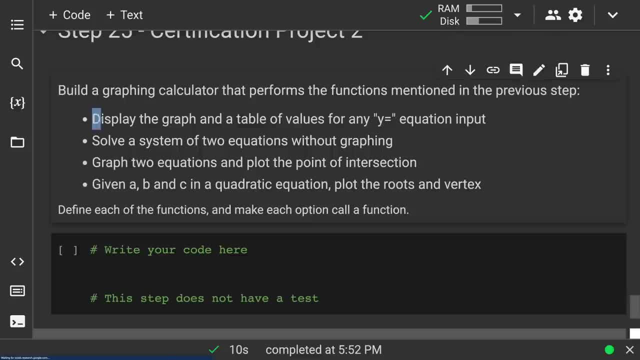 Certification Project To And You're Going To Display. You Know This Is What You Want To Do: Build The Calculator. That Is A Point Of. 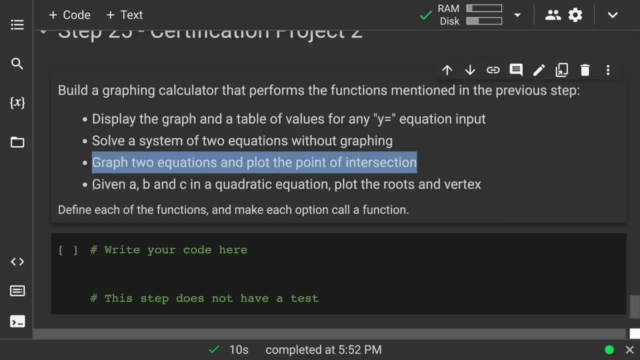 Intersection. So There We Go. That's Going To Be Pretty Big. You Know, Graphing The Two, Solving And Graphing, And Given A, B And. 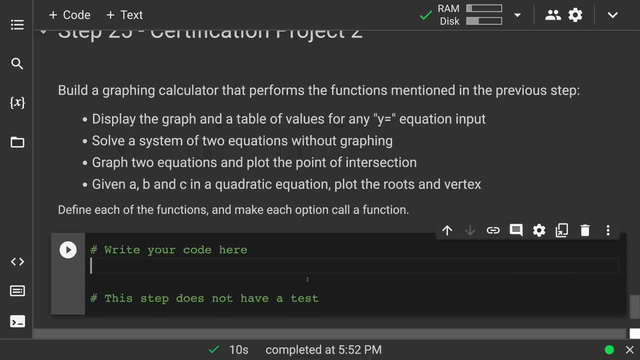 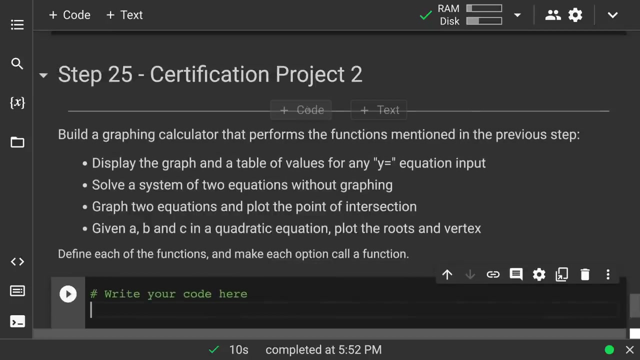 C Graphing. That Is The characters And A Graphing. This Is A Part Of The Code Of The Cake On The It's A Day. 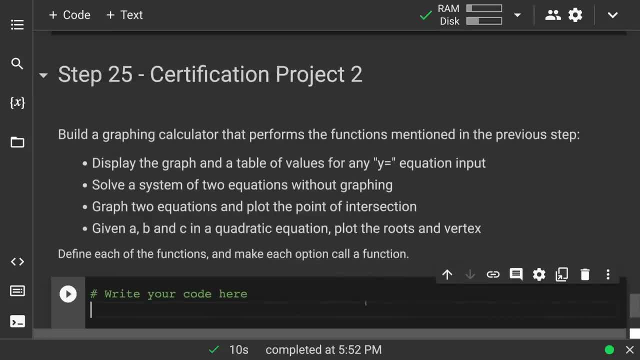 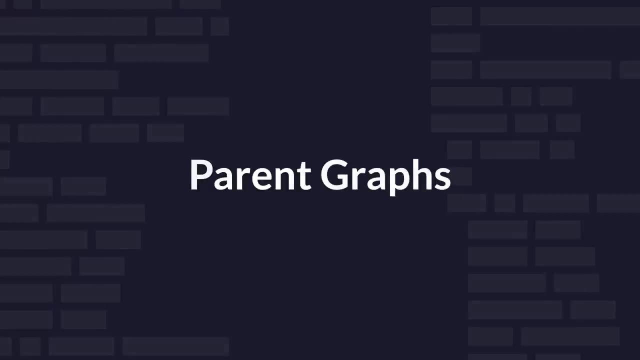 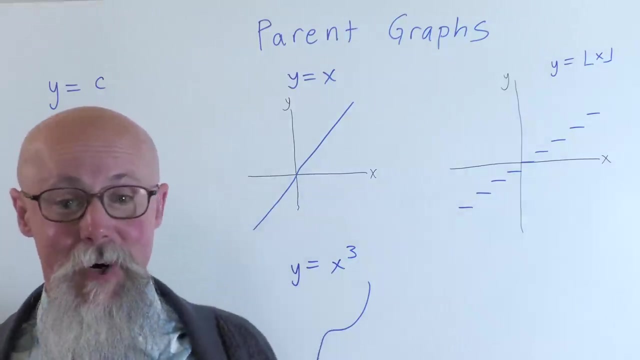 And Of The Work Of The, and we're about to then have some more twists and see some more complicated equations, some more. we can do with this, All right. So what do we mean by parent graphs? And you might have heard this in code: 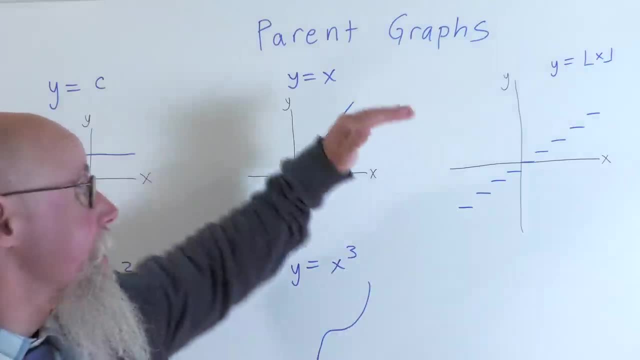 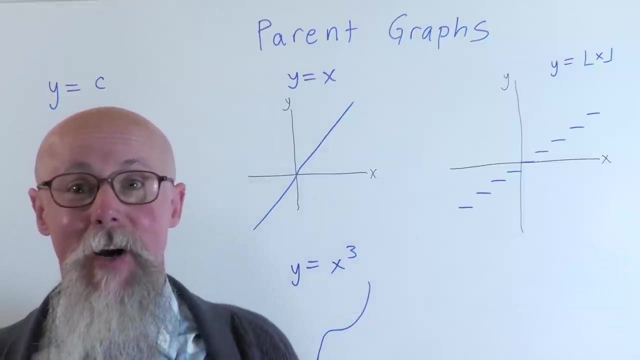 the parent or child, that the child graphs have everything that the parent graphs have, plus some other additions, And so these parent graphs are the basic patterns that other graphs then add to or change. So let's take a look at this. The most basic would be: y equals some constant. 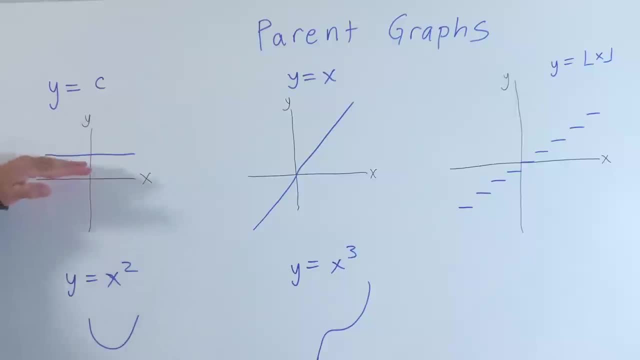 which I'll just call c here. And so that would be this blue line here, just a flat line, no slope, you know, like y equals three or y equals four, something like that. It could even be negative, but that's it. 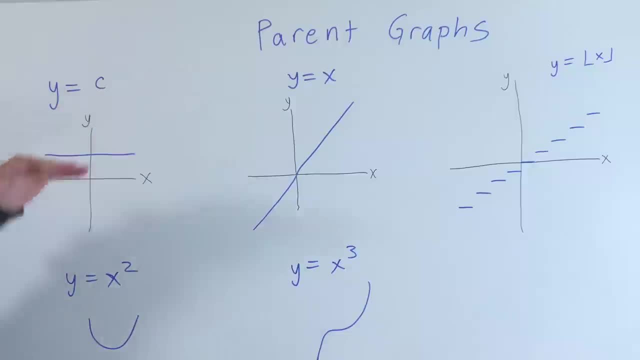 Nothing else And whatever. the constant is that graph's going to have that same look. you know: flat, no slope. you know nothing else going on. just y equals some number And that's why it's a parent graph. 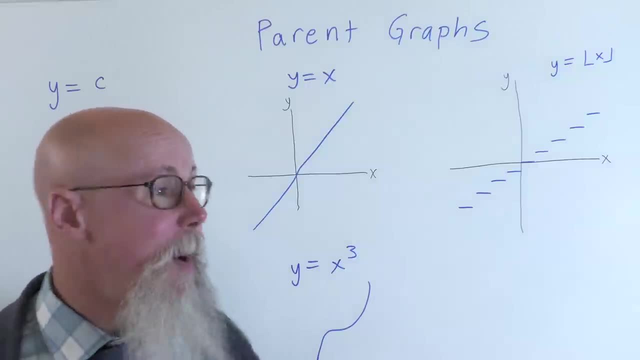 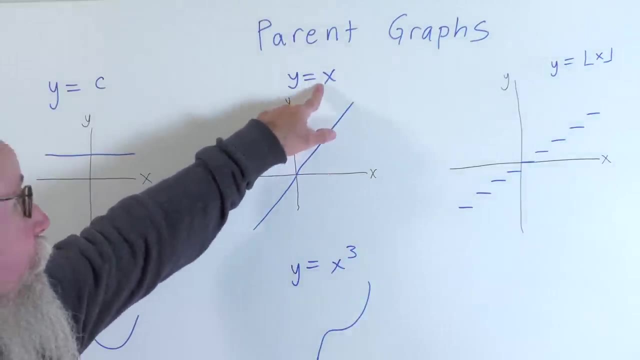 because that's like the basic pattern. Now we were talking about things like y equals mx plus b. Well, the parent graph for that is y equals x, just y equals x. So notice: slope is one, b is zero, And just that basic. 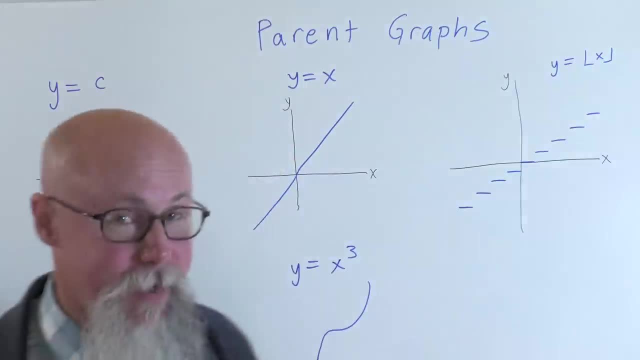 it's not y equals, it's a constant because there is a slope to it. But right, the paragraph is just y equals x, And then we can get like y equals, you know, 2x plus one, or anything like that. 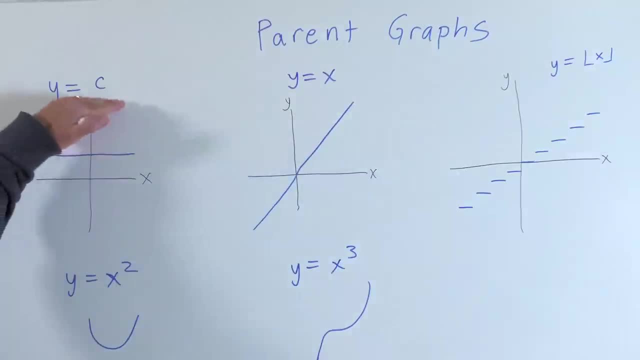 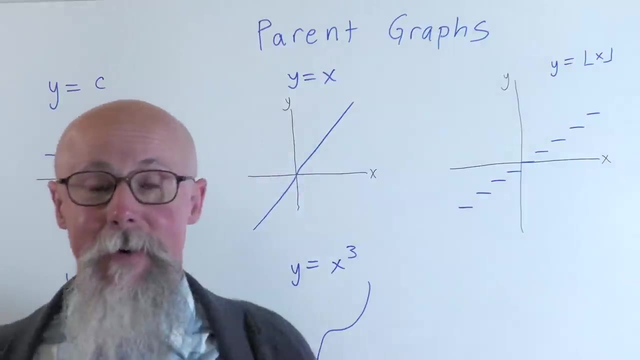 We can have other things, So this wouldn't add anything. This could add two things. You know, I have a slope, or I could have a different intercept, You know. so there we go. So that's the parent graph, Another one I wanted to show here. 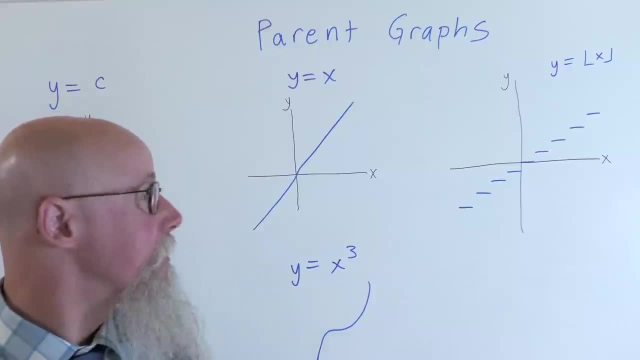 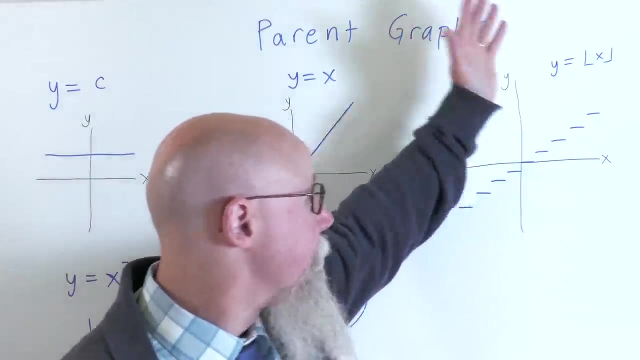 because I think the drawing of this works better than somehow, sometimes, how it plays out with Python. But this is the floor function, And so it's this step function. Some people call it step function, floor function, greatest integer, But the floor is when you're not rounding. 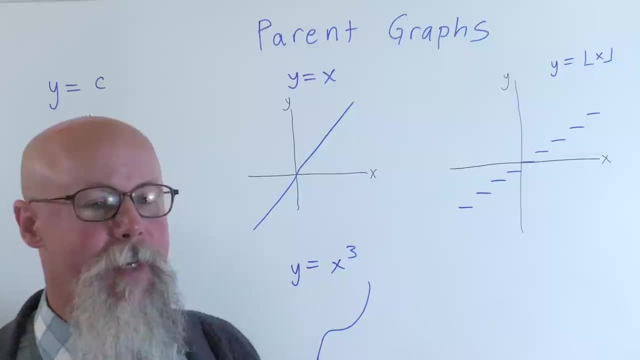 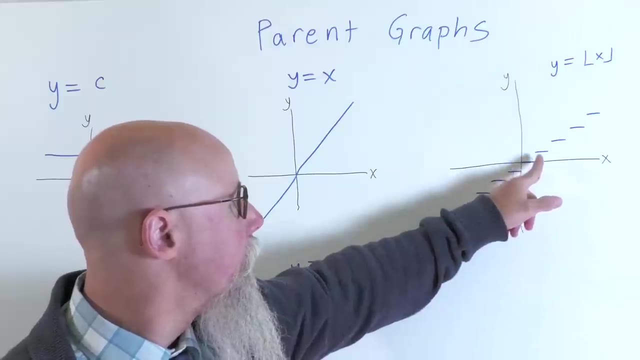 you're just dropping the decimals. Even if it's 0.9, doesn't matter. we're just dropping all the decimals, So it's the same value. So here, all these decimals, it's zero until I get to one. 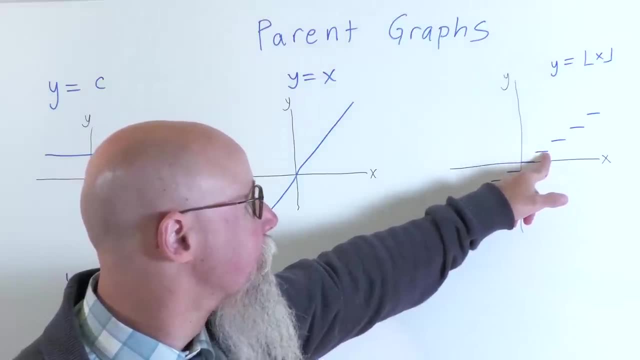 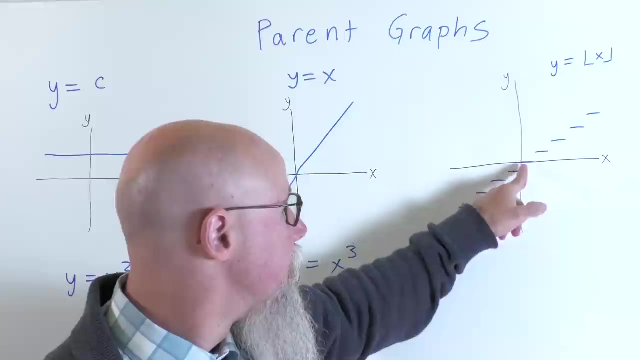 Now it's one, And then 1.1,, 1.2,. it's all the same until I get to two. So that's it. There are no in-between points here, It's just that integer. And then at the next integer it jumps up. 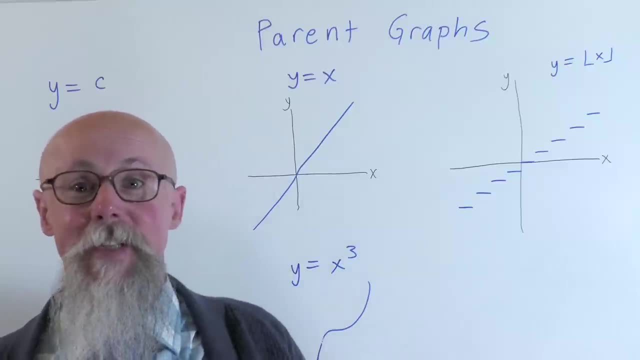 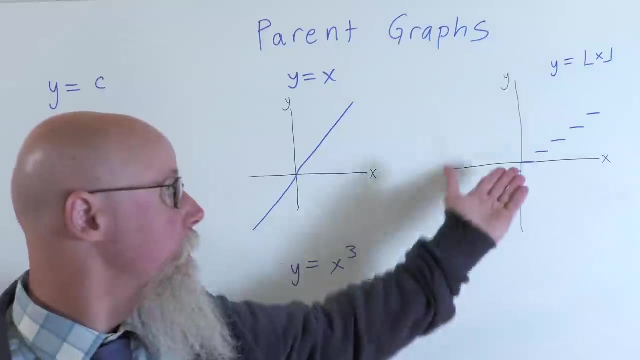 So again, that's a parent function And the floor function, the ceiling function- where, no matter what it is, I go up to the next number, or the round function. they're all very similar looking graphs, just shifted a little bit. 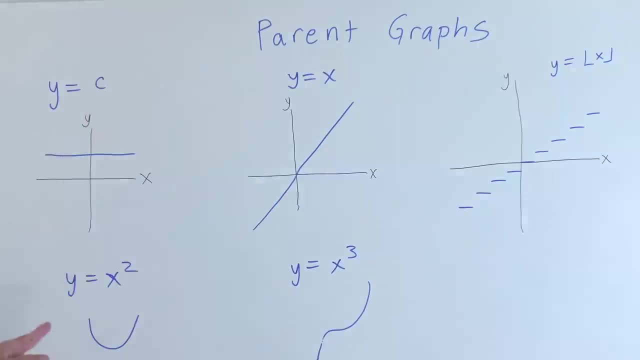 So that's why that's again a parent graph. We talked about x squared as a parabola, And I didn't worry about drawing even the axes for these, because I want to get the idea of this general shape. And then x to the third. 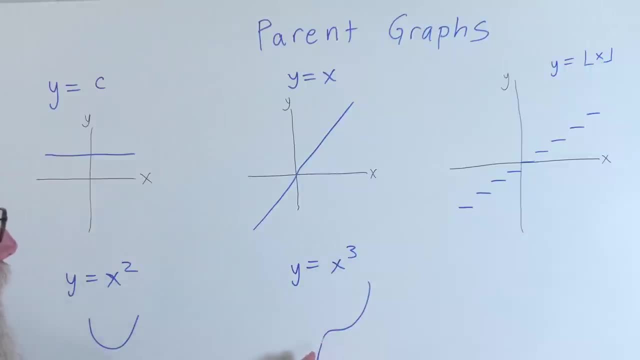 it's kind of like half this parabola bends down. Now, the reason why I just have these is because, as you get into x to the fourth, x to the fifth, all the even exponents, if it's just the parent graph- 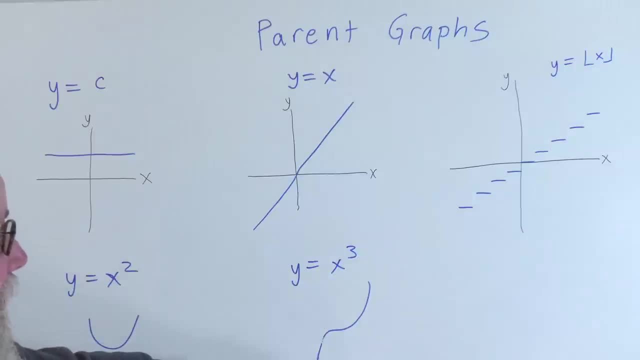 look more like this, All the odd ones look more like this. But then if I have other things going on in that graph- so remember, x squared could have ax squared plus bx plus c. Now, if I had other things going on, it's still a parabola. 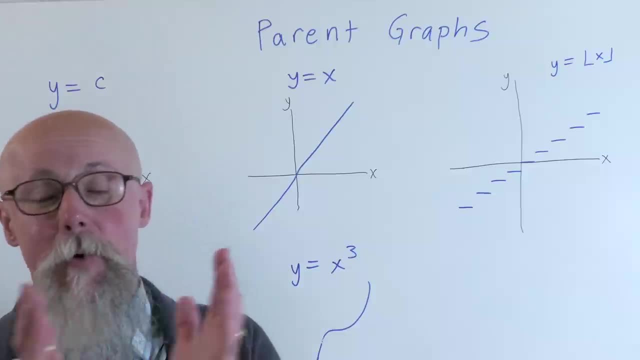 but it's a little bit different shape parabola. Maybe it's like a little bit narrower or a little bit wider or it's moved somewhere else, but it will still be a parabola: The x to the third, if I end up with x to the third. 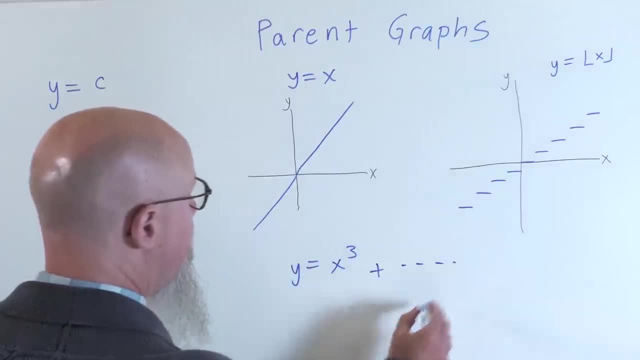 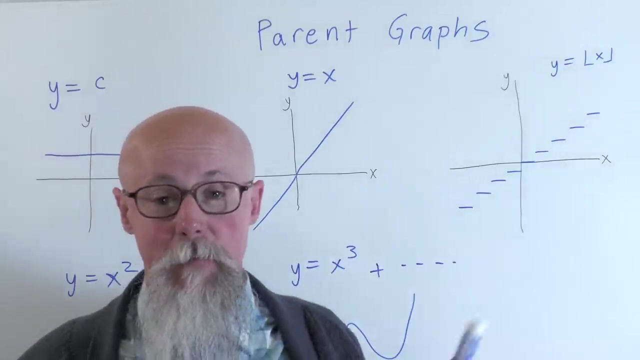 plus other things in there. then those curves, those get a little bit deeper. That's again paragraph. and then beyond that we get some other things, And we'll take a look at some of this in the code too. And the same with if I had x to the fourth. 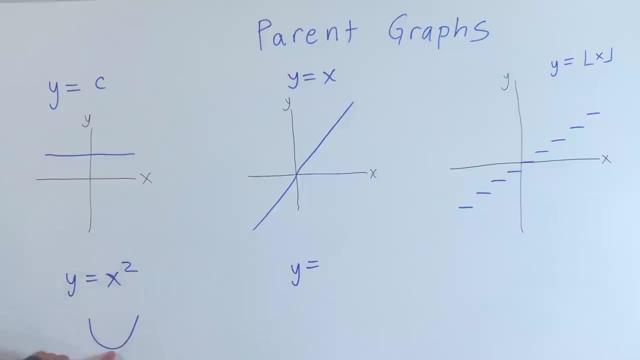 So x to the fourth is going to look more like this, maybe a little flattened in the middle. But if I had x to the fourth plus a bunch of other things in there, plus 3x, squared, something else, times x, all these things. 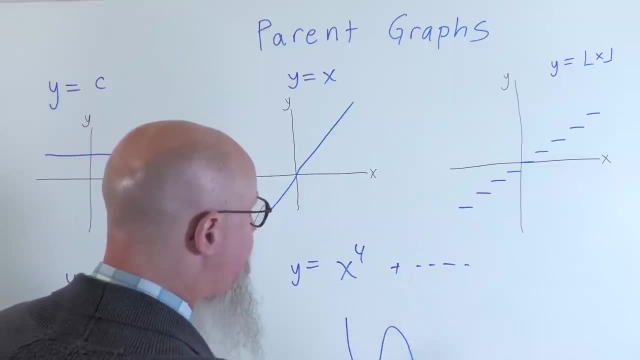 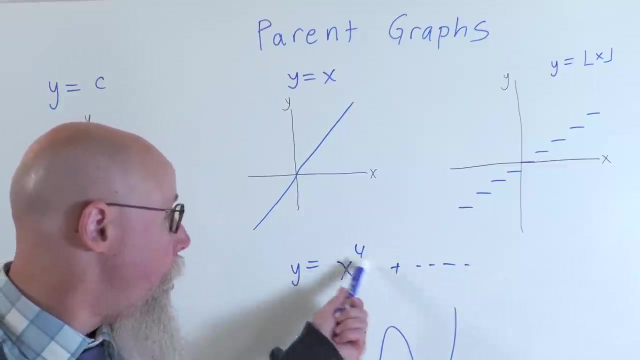 all these other things that could have three turnarounds at the most. You know, x to the fourth could turn around one, two, three times And you know, might not be always perfectly symmetrical, but if all the exponents are even. 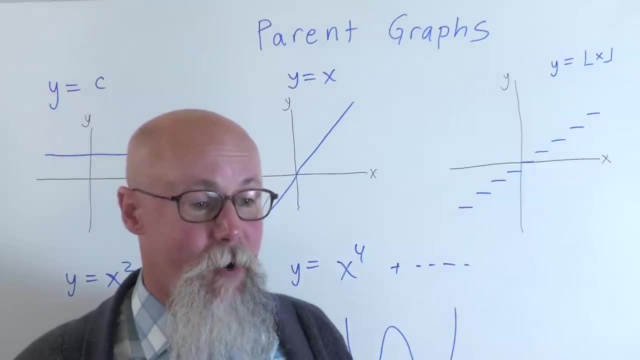 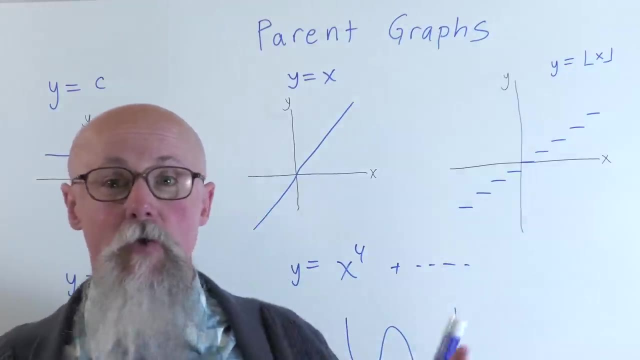 then it actually would be symmetrical. Kind of cool how it works out that way. So these other graphs, we have the paragraph, but then we could have other things going on, And I didn't want- I didn't want to draw a lot of this here. 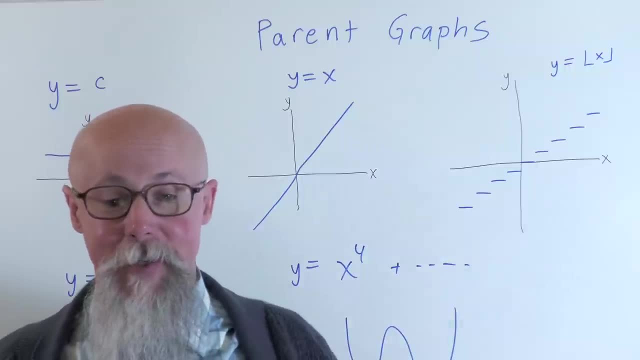 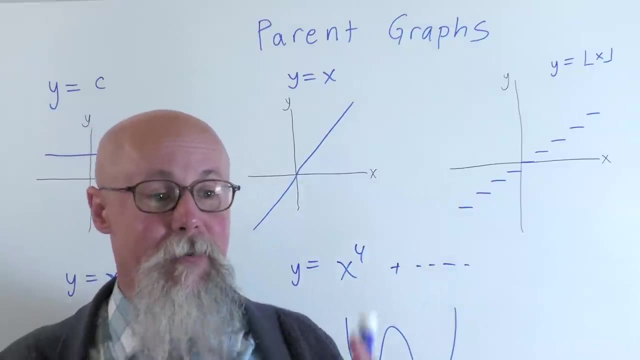 because I want to talk mostly about it when we get to the code, because that way we can see the graph and the way Python displays the graph is going to be much better than my drawing. We get the sense of the parent graphs. These are the basic patterns. 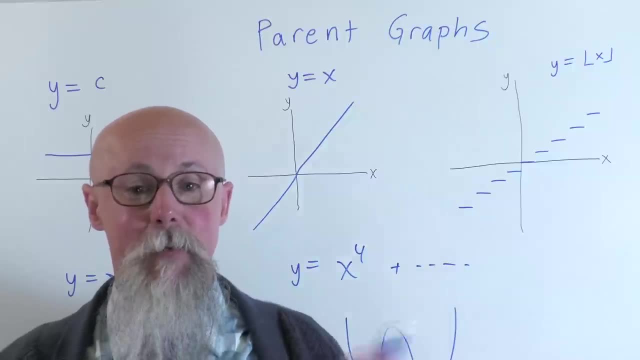 the simplest pattern of that type of graph And then we can look at what else we can change or add to each function and then how that affects the graph. So let's take a look at the code. So here we're going to look at all the parent. 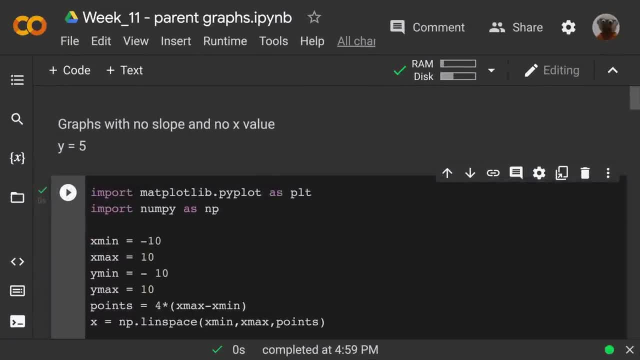 the parent graphs and the code to create them, And they're all going to start out with the same setup we've had so far for setting up any plot: matplotlibrary numpy: set up our dimensions, our points, set up the graph. 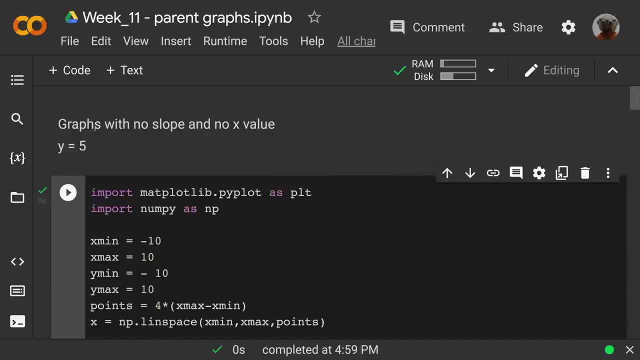 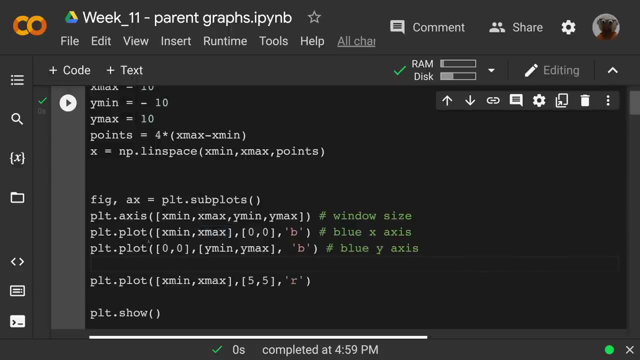 So this simplest one is just a constant: y equals five. or if y equaled any constant number- Notice x is not even in there- Just y always equals five. So when I plot this in the same way that I'm plotting the x-axis, 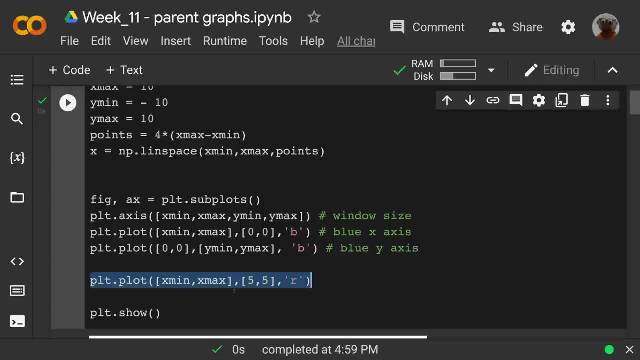 I'm just going to have this plot from the minimum to the maximum, And then y is just always going to be five. In this case, I'm going to make it a red line, And that's what it looks like. It's a flat line. 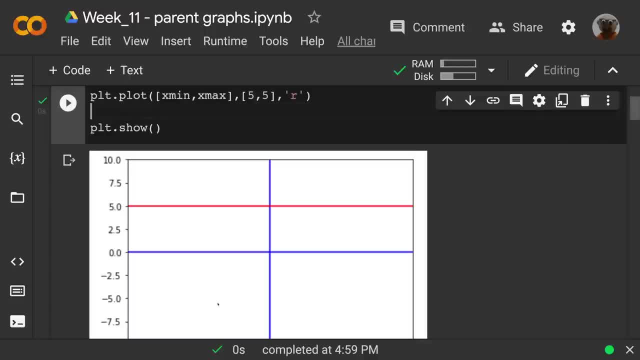 There's no slope because I don't have that whole part of the equation. No x-value and y is just always five, And it would be the same if y equals 7.5, or if y equals two or anything. Flat line, no slope. 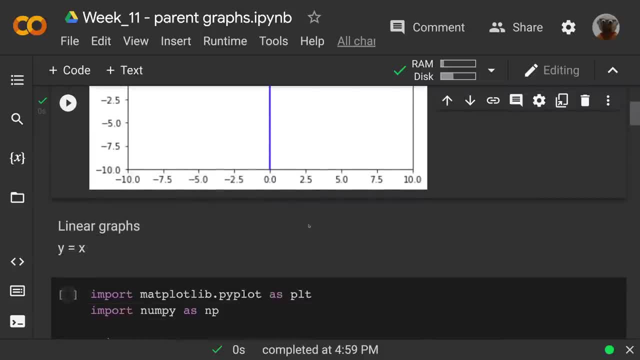 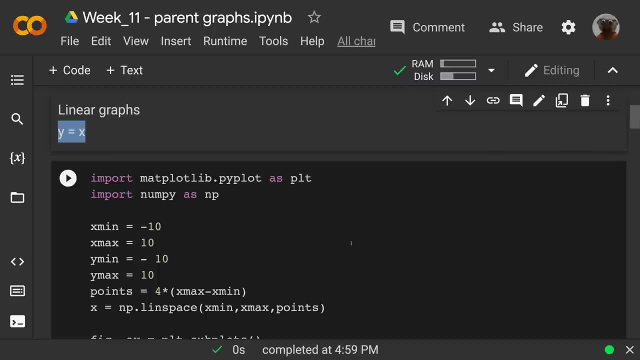 So that's a constant graph. And then the linear graphs. we were talking about linear graphs, but this is the simplest linear graph: y equals x. So anything else I do with that. You know I have a slope In this case. 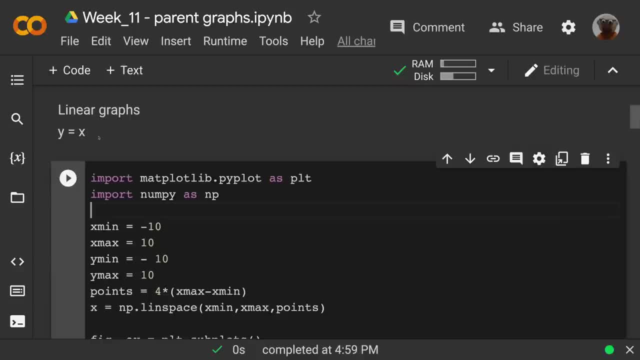 it's y equals 1x, so the slope is one plus zero, so the y-intercept is zero. Again, the simplest. And then anything else I do to that is an offshoot of this parent graph. So there's our simplest. 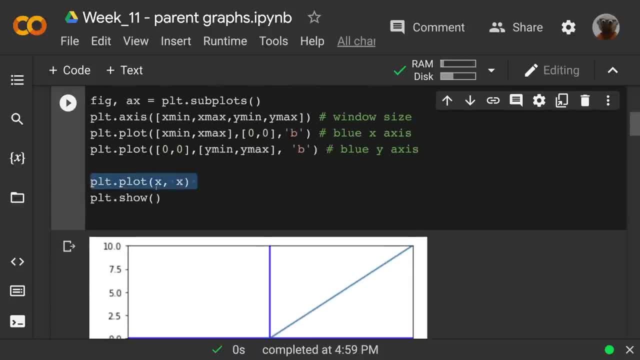 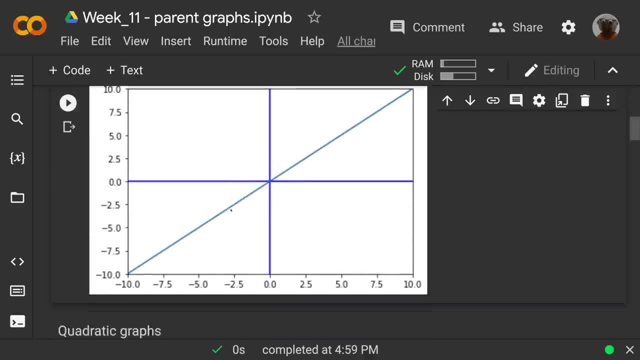 And notice everything else I do to set this up And how do I plot it. My x-value and then the y-value is x. So there we go, x, x And there's my. y equals x. graph Slope is one. 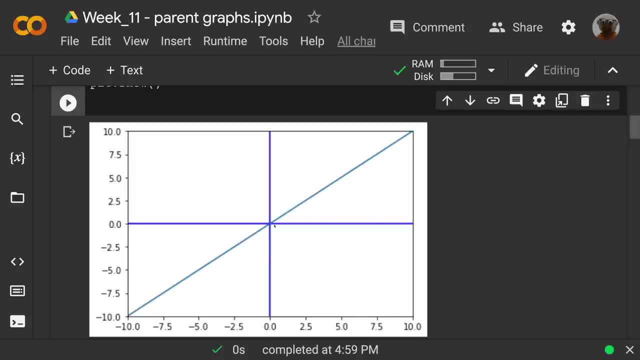 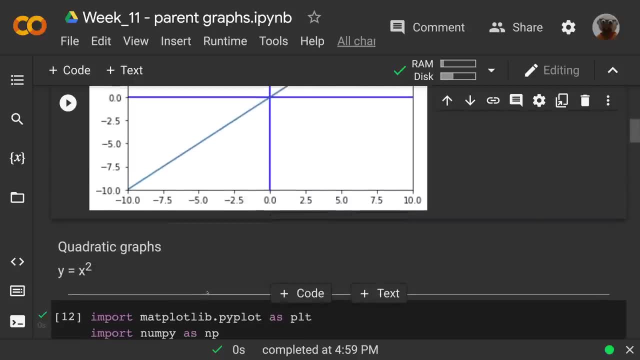 and it just goes on a diagonal like this. There we go. So every point here, you know 3,, 3,, 4,, 4,, 5,, 5,, etc. So the quadratics, We were looking at quadratics. 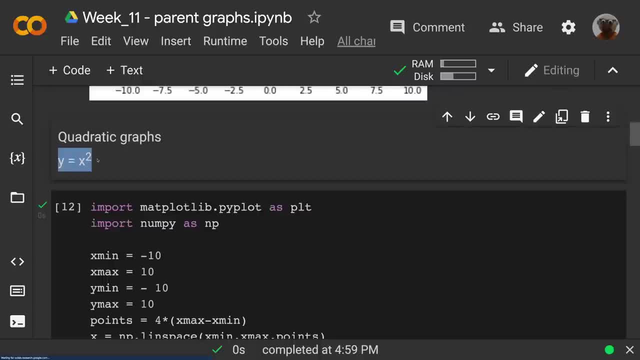 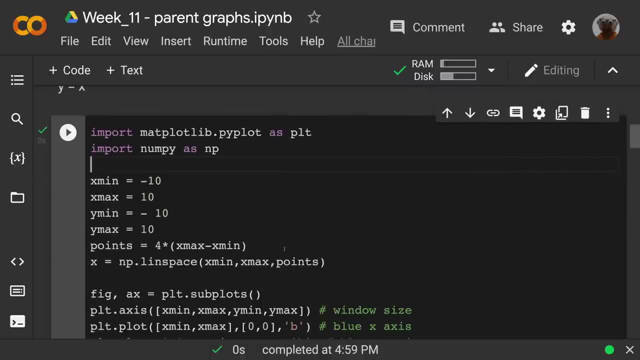 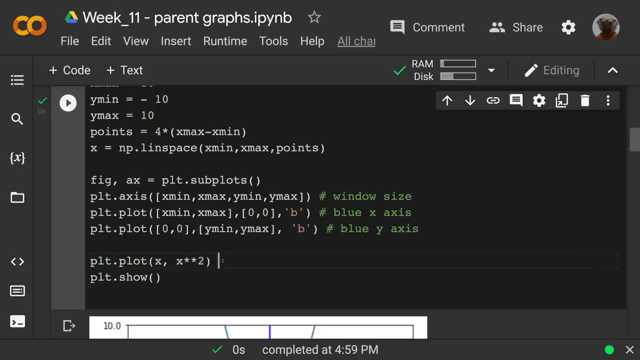 This is the basic quadratic graph: y equals x squared. So before I do anything else to it, that's just enough to make it a parabola. And here we're plotting this: My x-values, and then the y-value is x squared. 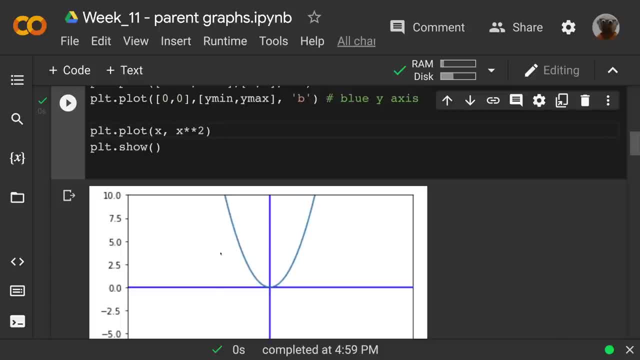 And there we go, Our parabola. So in this case you know x squared, so a is one, b is zero, c is zero. that's all we have, And then any other thing we do to the x squared. 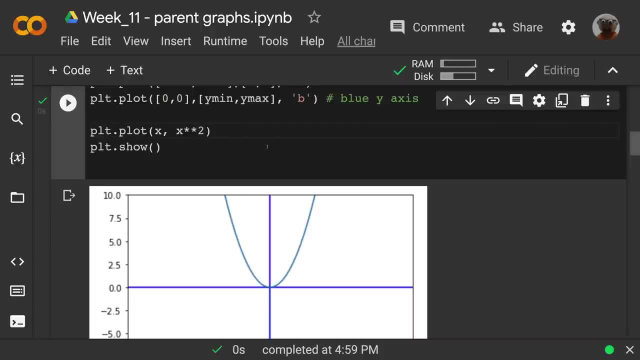 you know, add other things: x squared plus, you know, 3x plus 4, or something like that, or some, you know. whatever else we would have is an offshoot of this paragraph. So there we go, and I can make it negative. 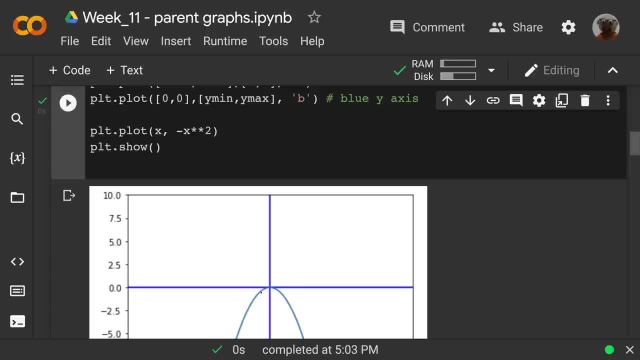 and change that And we see the negative. a flips it upside down. so we have, you know, negative like a frown, positive like a smile. So I'll go back to the smile. There we go Again. the basic, paragraph x squared. 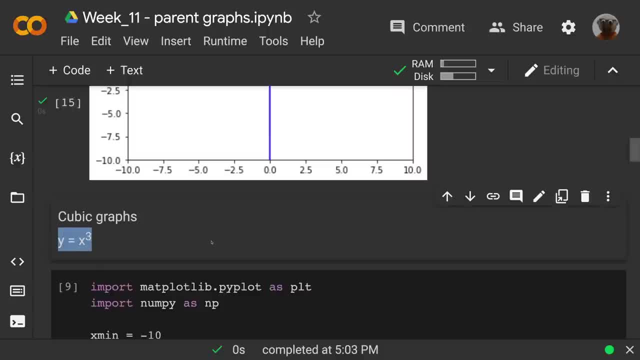 and then a cubic graph. y equals x to the third. So the quadratic is x squared because it's like the area of a square, if I know the sides. The cubic x to the third because it's like the volume of a cube, if I know the sides. 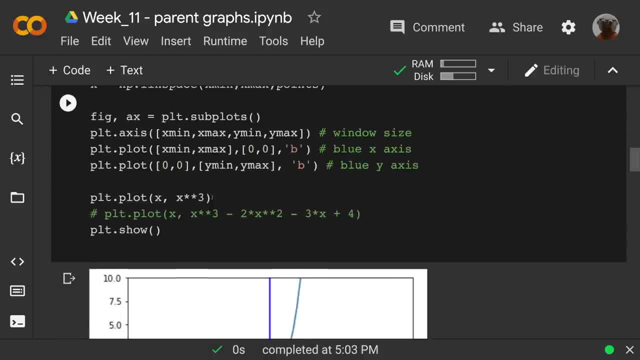 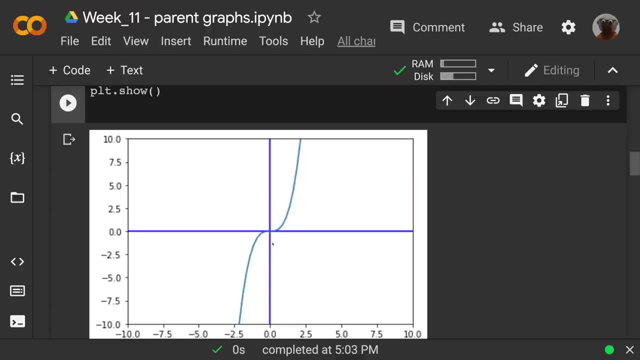 So setting up the graph here and the comment we'll talk about later, just starting out with the basic x to the third, And we see the graph looks like this. So you know some of these, you know I could sketch it out enough to show you. 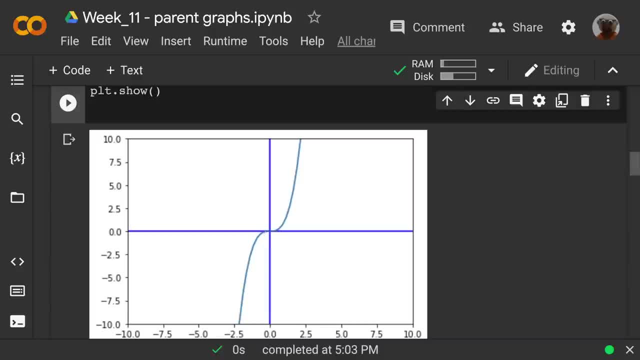 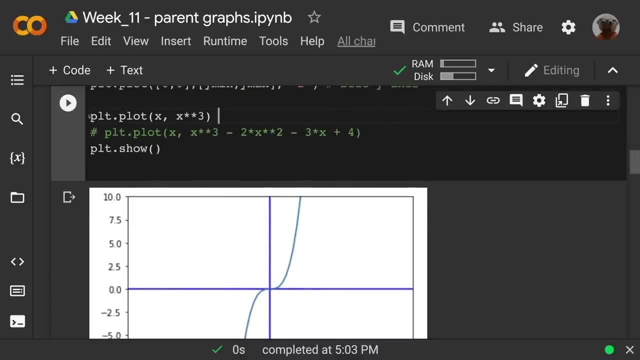 but we see it kind of looks like a parabola with the left side flipped down, but not exactly. And this is the simplest cubic graph. So what I wanted to show you is also supposing. we have supposing. I just have other things. 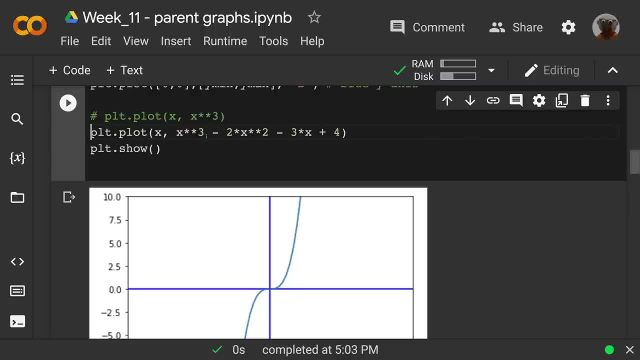 So plot the x values and supposing I had like x to the third minus 2x, squared minus 3x plus 4.. You see I can have all these other things going on in the graph And this is how it affects the cubic graph. 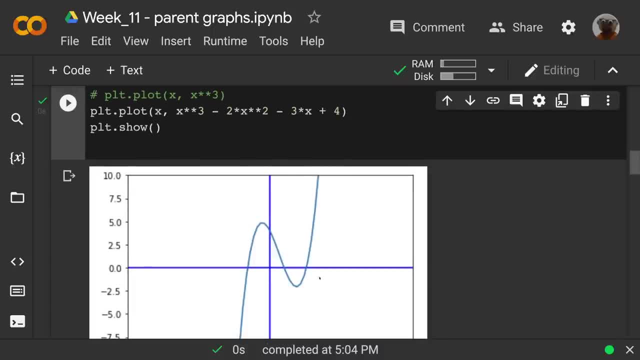 You see, it gets these deeper turns that were just kind of flattened out before. But x to the third is going to turn around at the most twice. So there we go. We see these possibilities here, All right, So again, you know. 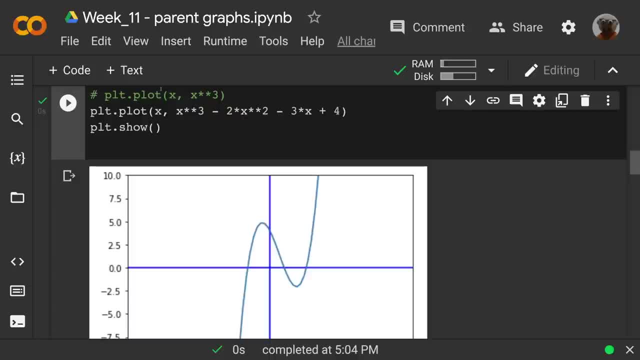 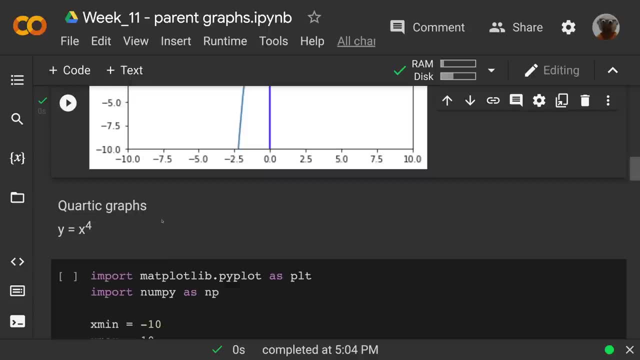 now, this is not a parent graph. This is, you know, a more complex graph. The parent graph still is x to the third, So we go x to the fourth. And, yes, they have a name too quartic, So x to the fourth. 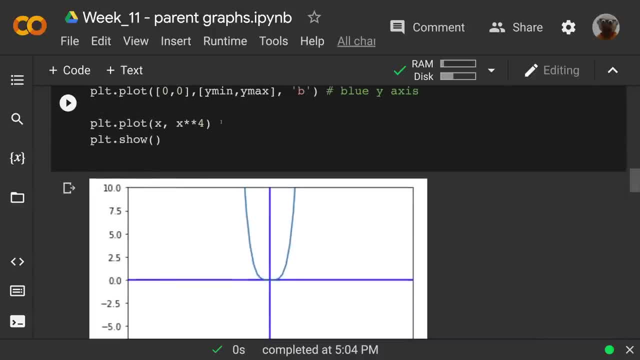 And all of our even exponents. So we see I'm just plotting x to the fourth. All the even exponents look a lot like this. So x to the fourth. If I also had like x to the sixth, notice how it's similar. 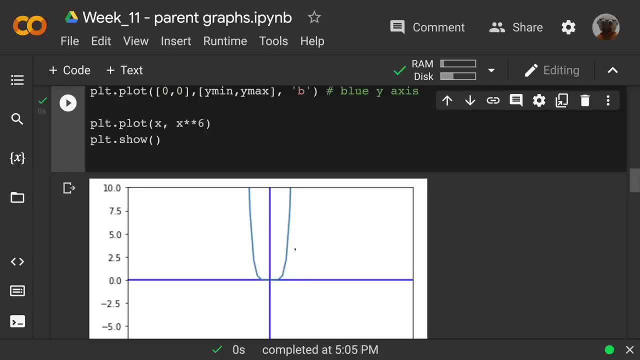 And I probably need more points to make this look smoother, But you get the idea. Now this, this is where it gets beyond what I can graph, what I can draw, So I like showing, showing it with the code. But all these, 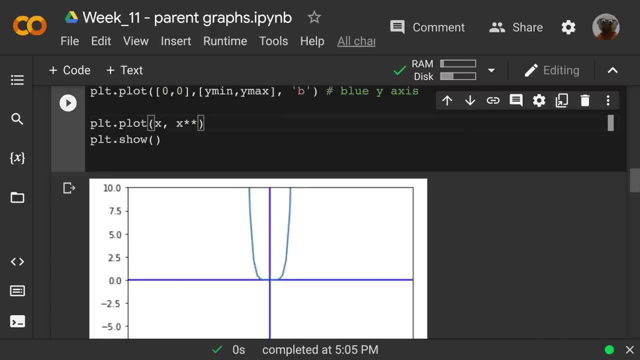 even exponent graphs. we might be able to do x to the eighth and it might look horrible. Eh, that looks kind of horrible. So x to the fourth is probably the last good one. Other than that, then we have to change. 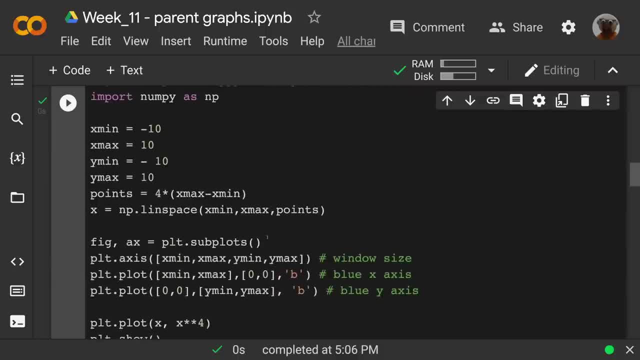 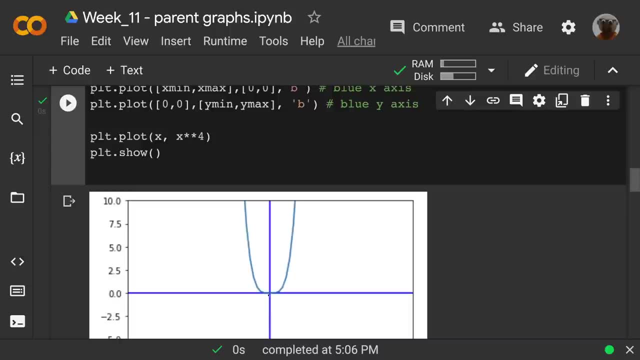 you know how many points we're doing to really make it a lot smoother. But that's where it kind of looks like a problem. It just flattens out more around zero And all of the even exponent parent graphs will look like this: 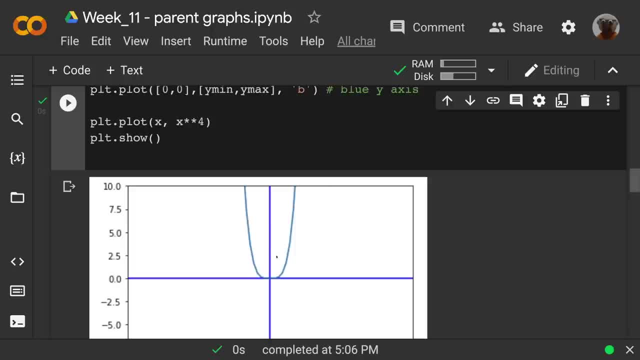 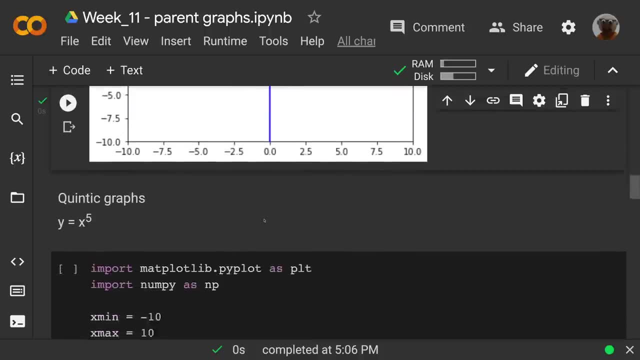 And I also could have x to the fourth, plus other things, and then the graph would look totally different. That could go up and down as many as three times. I could have as many as three turnarounds And quintic, you thought we were going. 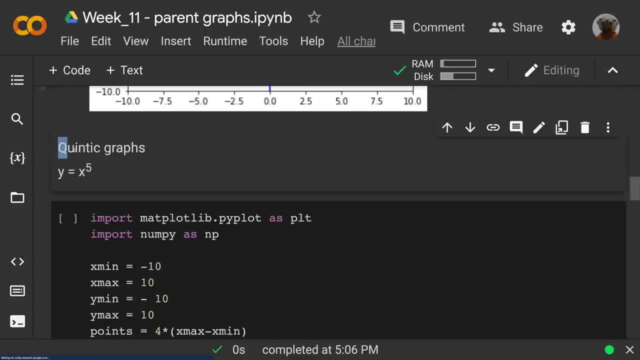 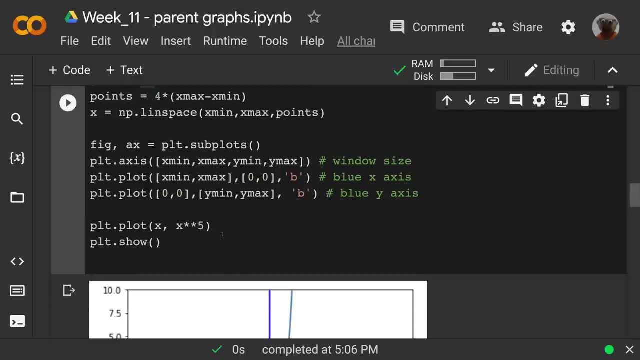 to run out of names. but nope, x to the fifth. we have a name for that: Quintic, All right, So x to the fifth. and when we look at this, there we go. x to the fifth looks a lot like. 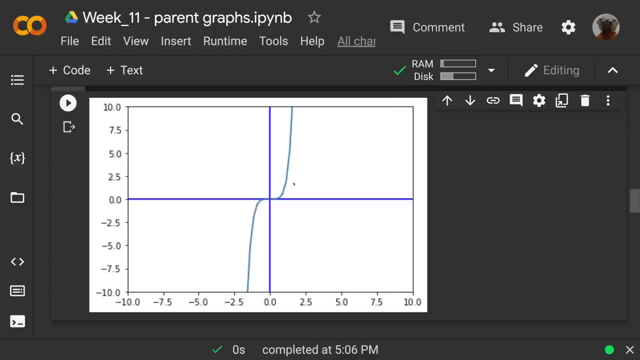 x to the third. So all the odd exponent graphs are going to look a lot like this, But again just a little bit more flattened out. And if it's just this, if I have x to the fifth plus other things, then the graph could be: 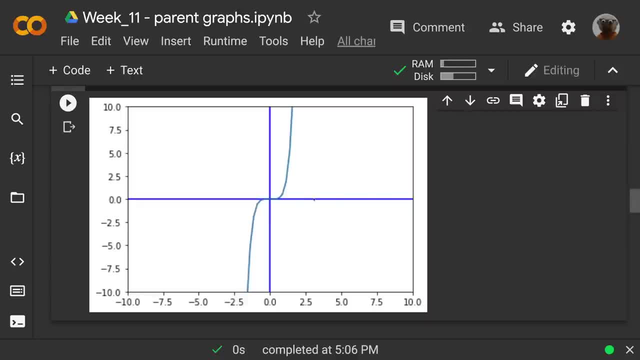 all over and it could turn around as many as four times. But there we go. So all the even graphs are like x to the second or fourth. It's symmetrical about the y-axis and kind of looks like a flattened parabola. 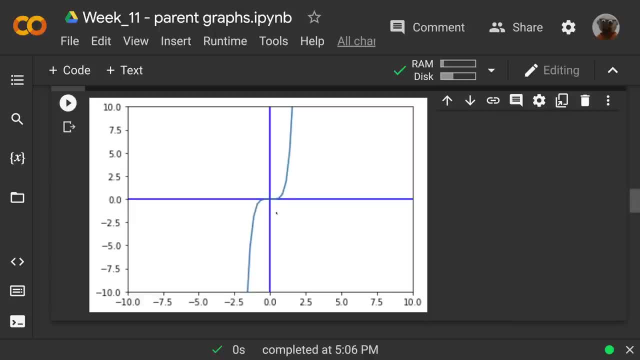 All the odd graphs look like this: x to the third, the fifth, all the odd numbers look like this, you know, and it would go back and forth And then with you know, as they get more complex, with other things going on. 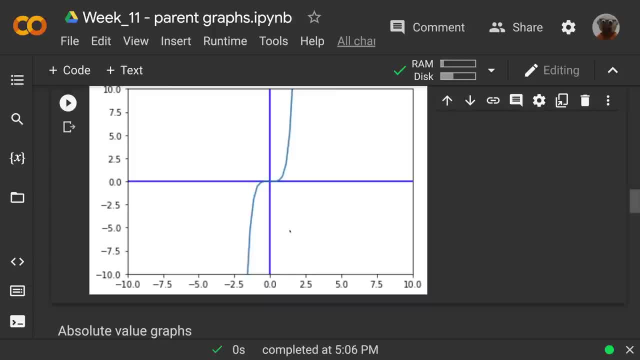 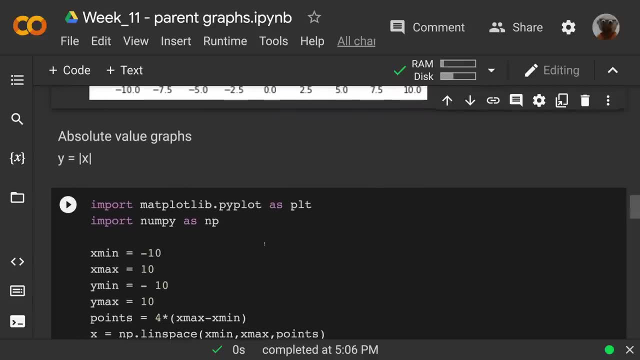 you know you're getting beyond the parent graph. then we have all the. they can actually have the ups and downs. So the absolute value graphs, and there's a lot of patterns with absolute value graphs that are also the same as they would be. 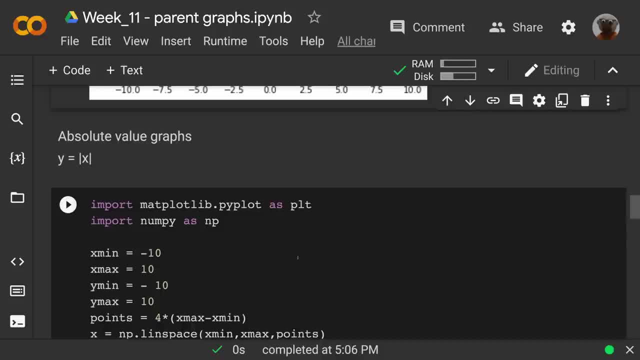 for x squared graphs the way the vertex can move around. So the simplest absolute value graph is just this absolute value of x. But like the other graphs, I could be multiplying by something here, inside the absolute value or outside. I can add or subtract something. 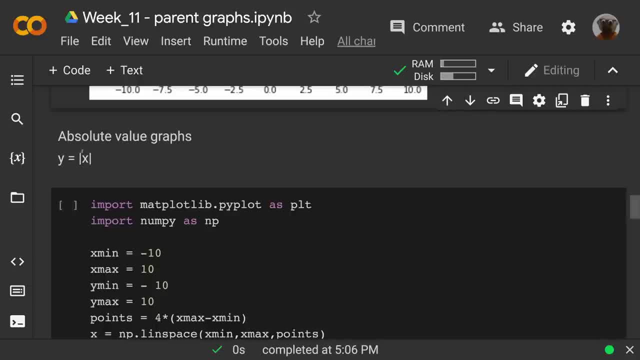 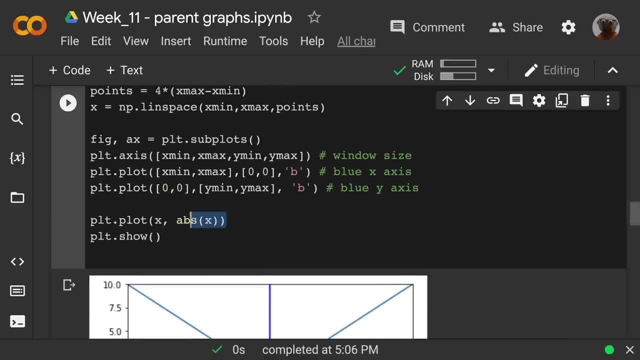 So this is how I would write absolute value, with the two vertical lines here next to it, not parentheses. And here's how I would put this in code ABS And notice I don't actually need to import anything. That's part of the 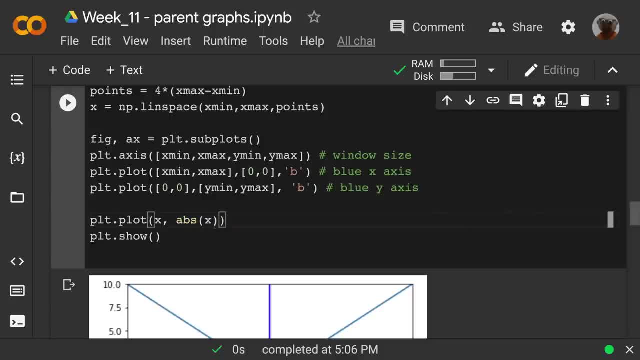 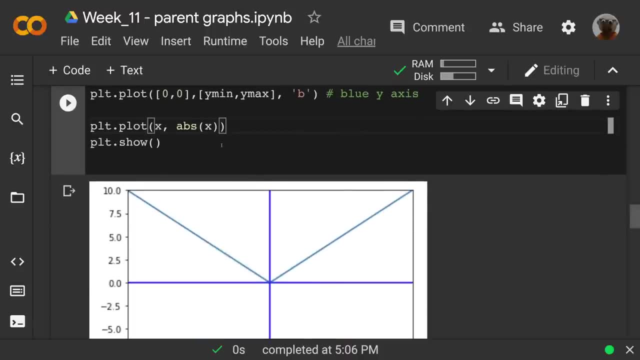 core Python library. So that's the absolute value of x. So as I plot it, then it looks like this: Because absolute value means it's just the number, like positive or negative doesn't matter, It's just the number. 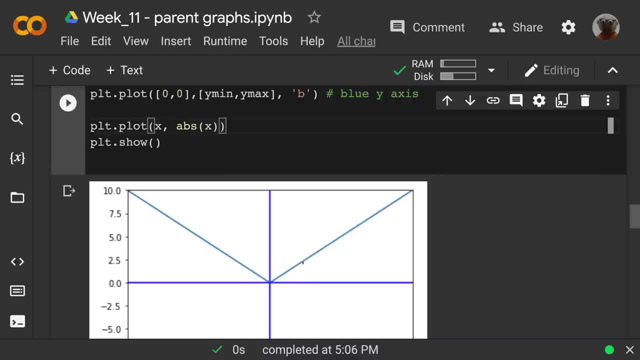 So it would be like plotting: y equals x and that would be in the positive direction, But y equals negative x. so for all these negative x values, the y value is positive because it's absolute value. So that's why, instead of continuing down, 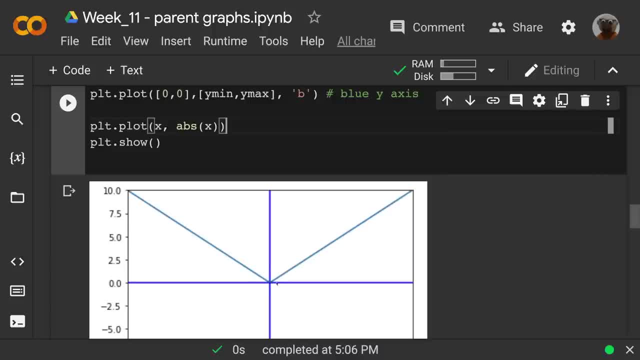 like the y equals x graph. it comes to a point and makes a v. So there we go. So just like x squared, whatever x is, it's going to, it's going to end up being positive when you square it. 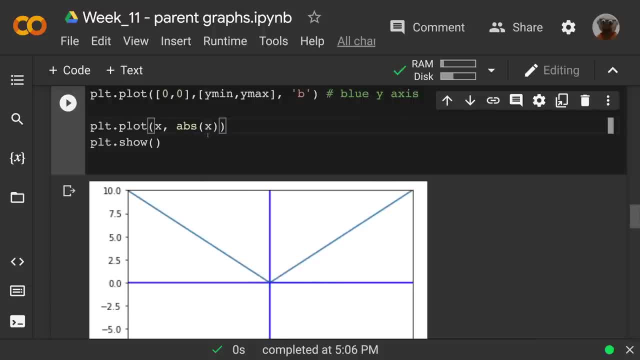 Absolute value just makes it all. it just doesn't do anything except make it positive, And so that's why there's similar patterns to some of these. But there you go, Perfectly straight lines, come to a point That's the absolute value graph. 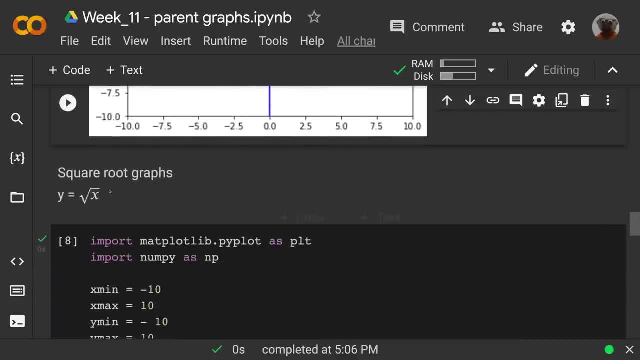 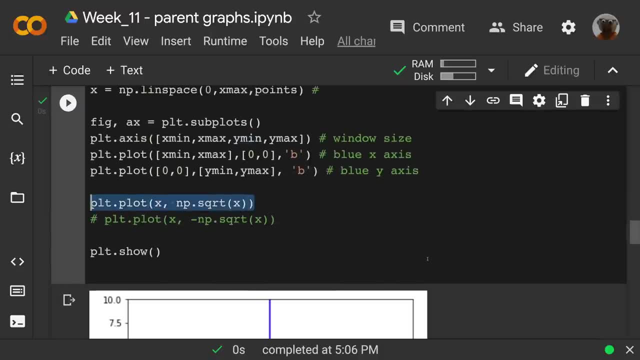 And then I can have square root graphs. There we go. So here's how I write the square root. if I was writing it out And if I'm plotting it, I'm going to use this. Now there's mathsquare root. 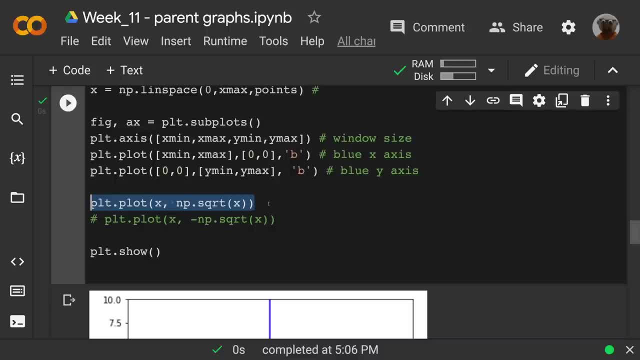 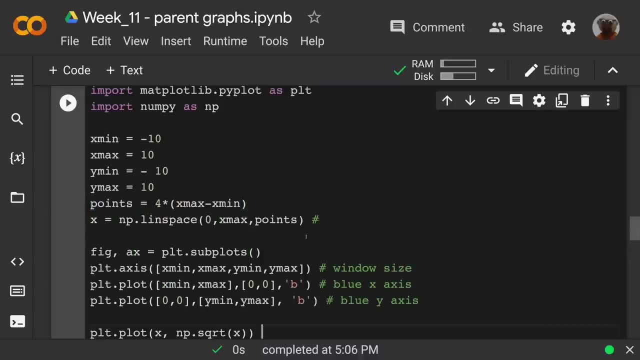 and other ways to get a square root, but I'm going to use numpysquare root because we're already using the numpy library for everything else. So, since I'm already using numpy for everything else that I'm graphing, I definitely want to use. 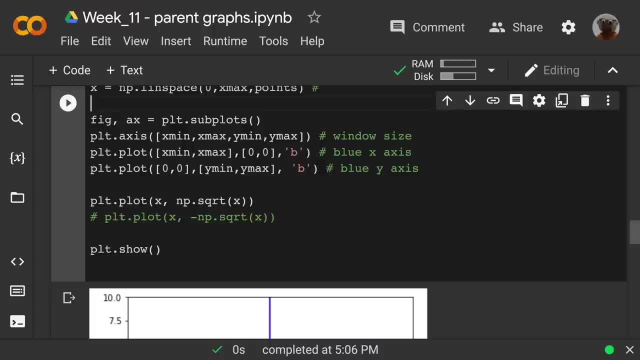 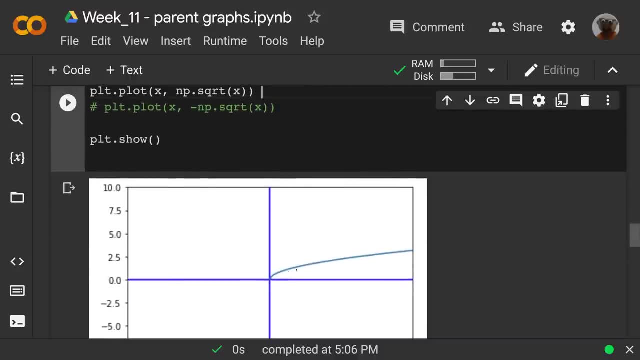 npsquare root. So the comment we'll talk about in a second, but here's the basic square root graph And we can start talking a little bit about inverse functions, because this is the inverse of x squared And that's why I also included this. 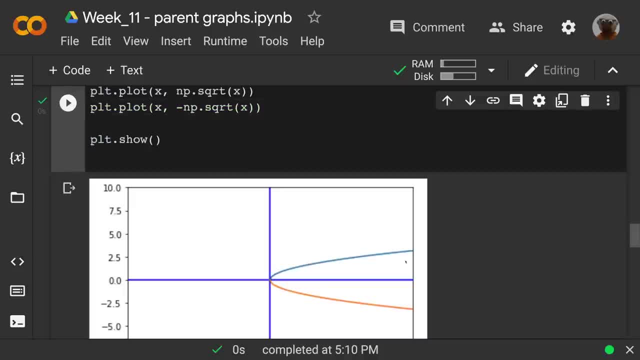 that if I uncomment that and now run it, you see now just the square root. it's just going to be positive, because if I include the negative part then that's not a function. These x values have two possible y values. 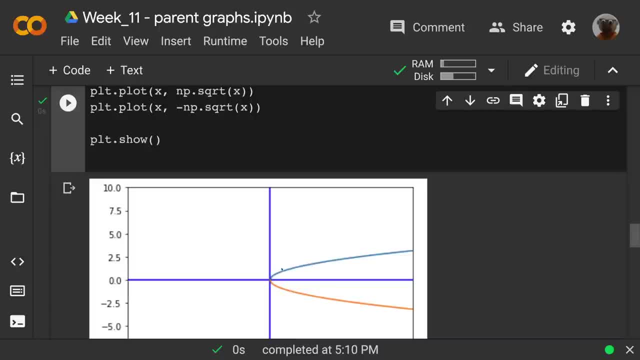 But when I put them together I see that it looks like a parabola on its side, And that's really what it is. That's the inverse of x squared, because I want to do the opposite as square root things. So 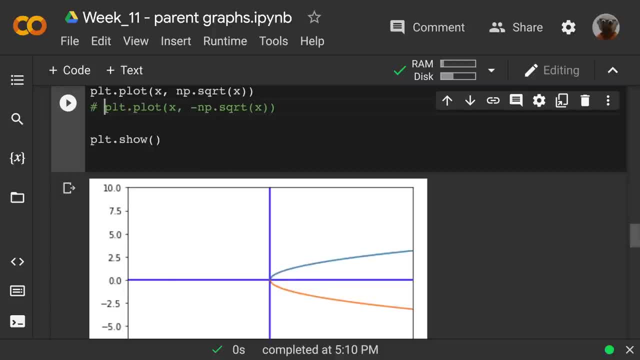 that just helps us see it, but the full graph, the true square root graph, is this, because then it's still a function: All these x values have one y value And there is just no y value beyond here, beyond this. 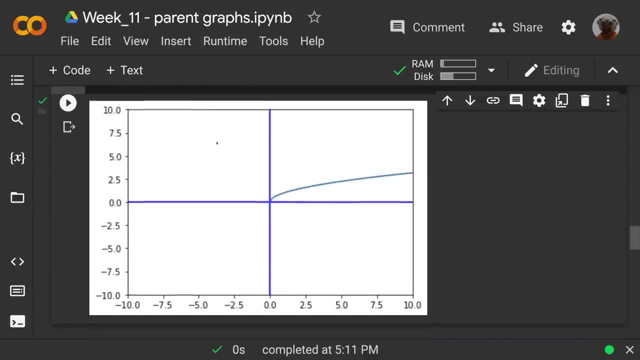 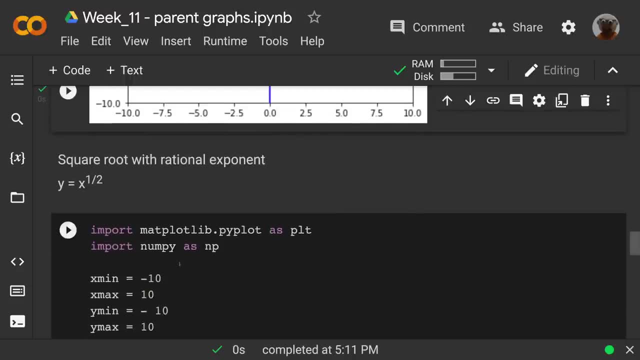 All right, so there we go. So there's the square root graph, And another way to do this is with a rational exponent. Now, overall for this, graphing Python does not like rational exponents, So I'm going to do this here. 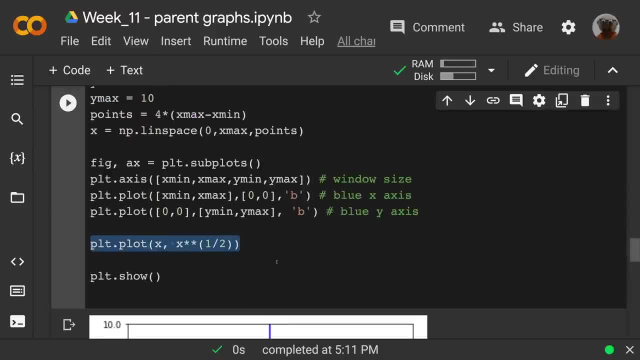 and I'm going to show you that this actually did work next to the one half exponent. But if you try this for any pretty much any other fraction instead of one half, it's just not going to work. It's just going to give you. 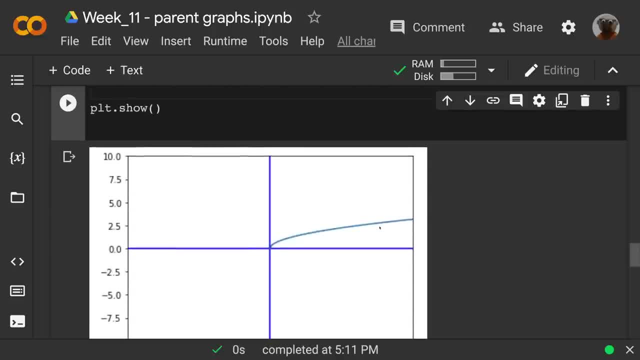 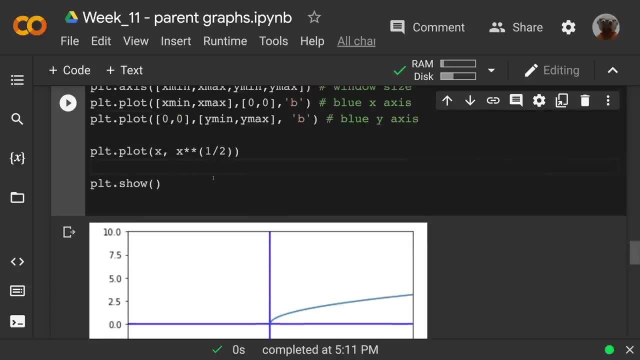 an error. Python doesn't like it. But there you go. That's the same graph. So x to the one half In solving it. if you weren't graphing it, you know it works out nicely. The denominator's your root. 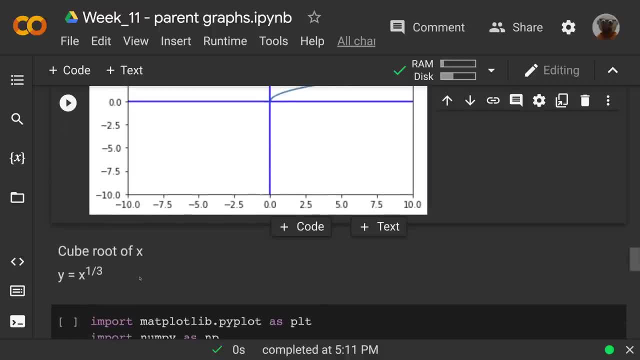 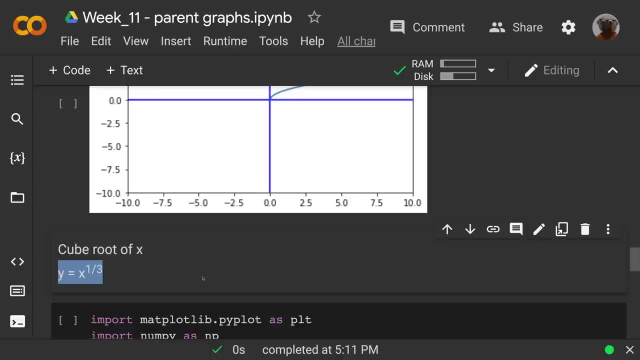 So, square root, denominator's two. Or if I had a cube root, the denominator's three. So I'm going to write it like this here: x to the one third. So that's the cube root of x. 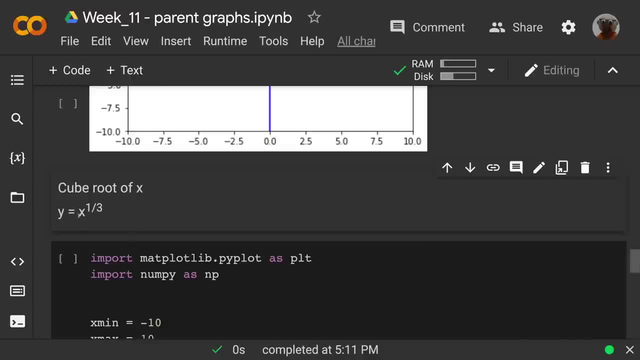 So it's what number times itself three times gets me x. So like the cube root of eight would be two, because two times two times two is eight. So we're getting the cube root and I don't need to worry about the rational exponent here. 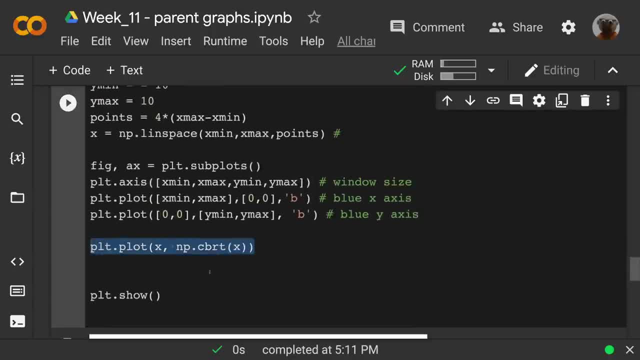 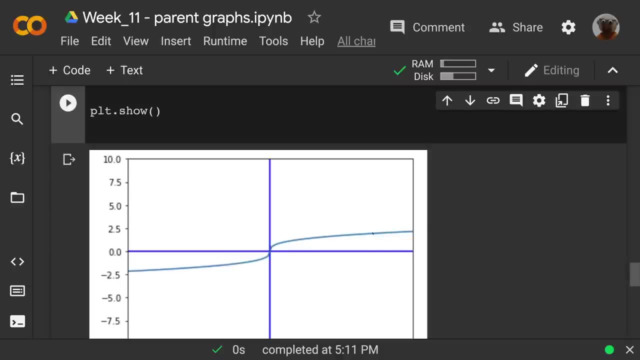 because numpy, just like there's a square root, there's a cube root also. So c b, r, t, So that gets the cube root And this one. I can have negative values because if the factor shows up three times. 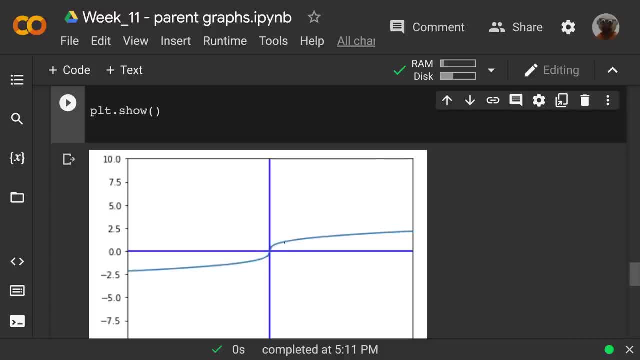 I can have negative, negative, negative, So that works. So there we go. I can get the cube root of x, There we go. So somewhere around here I have, when x is eight, y is one, There we go. 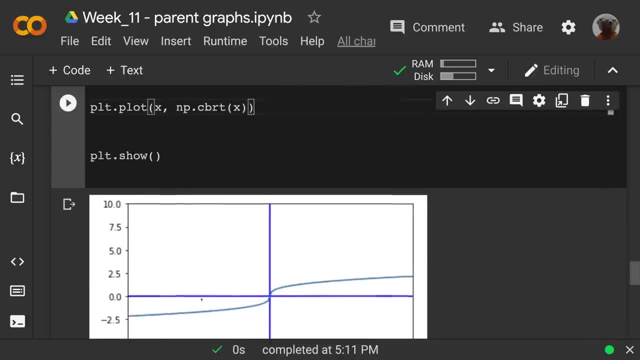 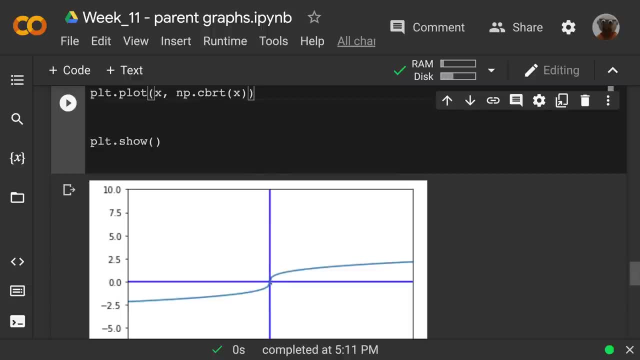 And then we get the cube root. So all these parent graphs, just like the other ones- I could have other things going on in this equation- The cube root of x plus something that would shift it up. You know, I can move it around. 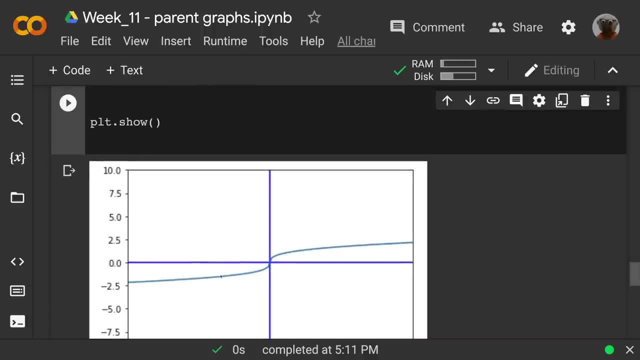 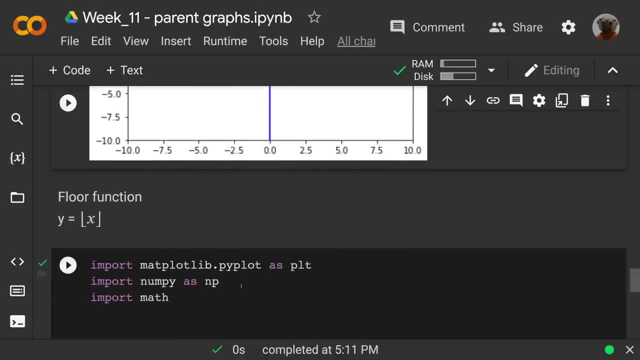 but these are the basic parent graphs, These types of shapes, and then other graphs are just versions of these. Alright, so the floor function. Now there's the floor. Notice, it kind of looks like absolute value, but it does have feet. 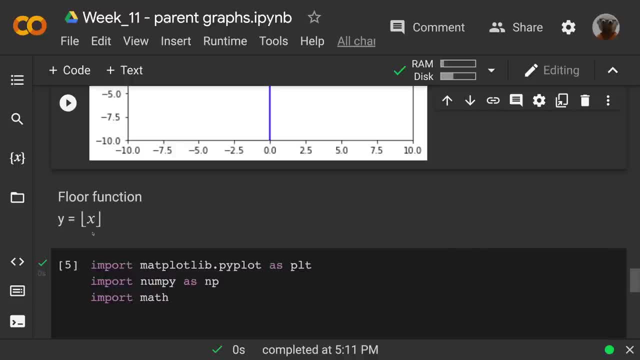 at the bottom that go underneath kind of like an L and a backwards L to show you the floor. The other function that's similar to that is the ceiling function, And the floor function is the one where you drop all the decimals. 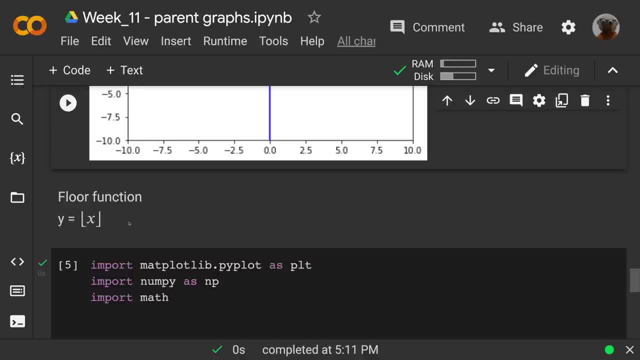 So it doesn't matter if it's like 5.9, and it doesn't round, you just drop it and the answer is five. The floor function just drops the decimals and just takes the whole number. Other than that, other times people call it. 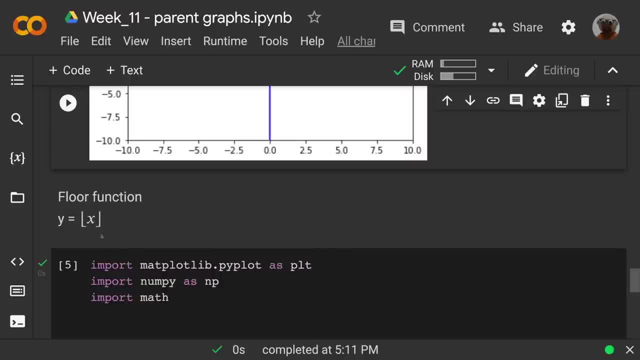 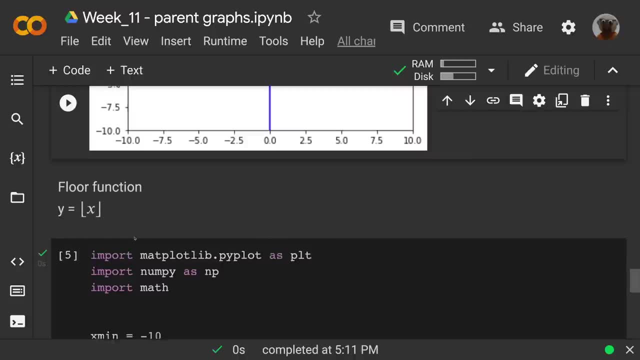 the greatest integer function or the integer part function- Same idea. There's also the ceiling function which, no matter what the decimal, goes up to the next one and we have round. they all work very similar. So we have all of these. 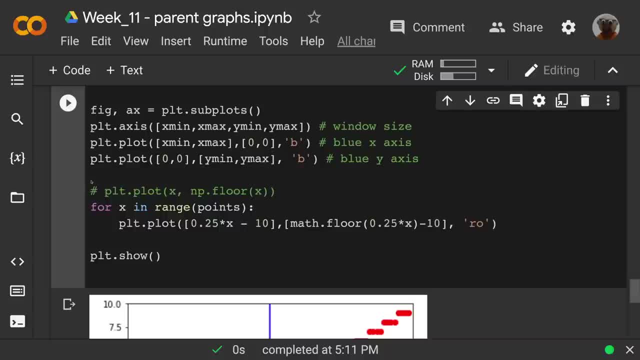 and to plot the floor function. now I want to show you this. This is actually a function npfloor, But there's a reason why I didn't do that. first, Because I put all of this in a loop to graph this. 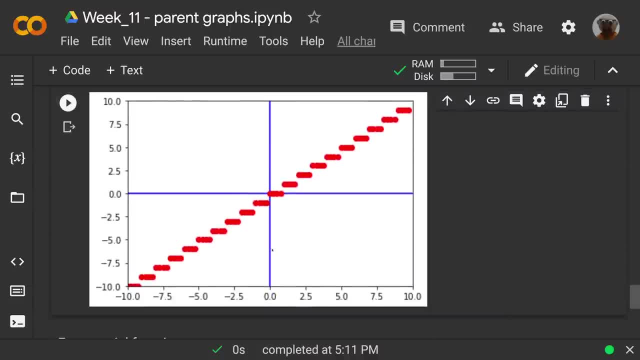 as a bunch of points, Because I feel like this illustrates the floor function a lot better. It does give these steps- and sometimes in the graph people call it a step function. So it's the same value until you get to the next integer. 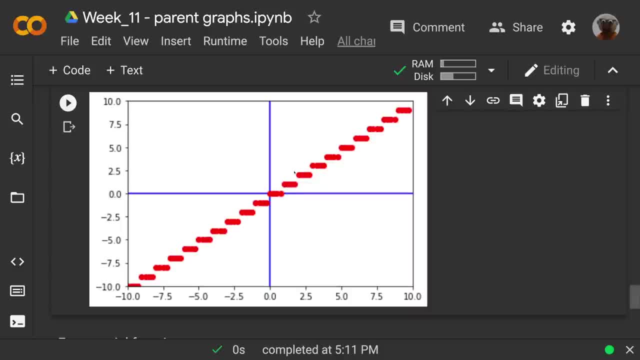 then it jumps up And it's that same value until you get to the next one next integer. so all these are just sudden jumps. once it gets to the next integer and it's the same value, it doesn't change, because if it was 3.1, the floor is 3. if it was 3.5, the floor is 3. 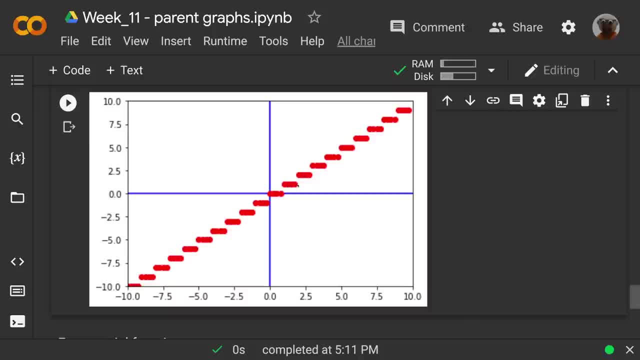 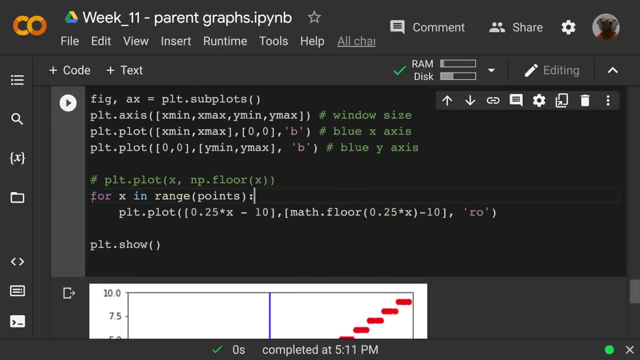 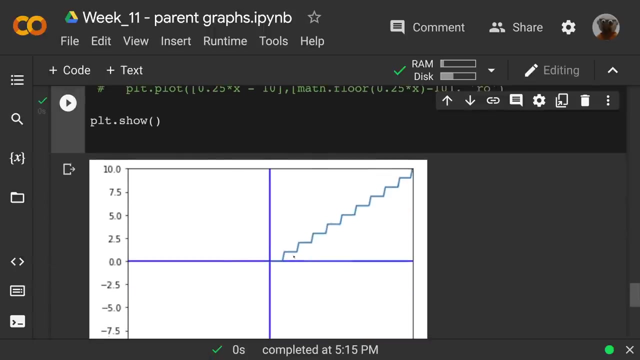 it's 3.6. you know all those values. if the floor is 3 and then when it gets to 4, boom, then it jumps up. so the reason why I went through all of that is that the actual floor function I feel like doesn't display well, but I'll show you. you see, it gives these values. 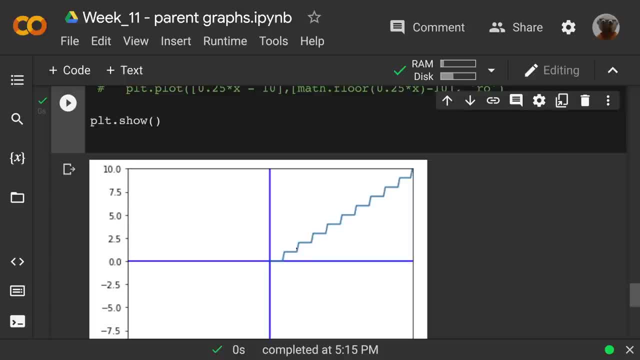 but these vertical lines really shouldn't exist because it's not continuous like that and so it's just. you know, numpy just wants to connect it. but that's what the floor function looks like in numpy, but truly mathematically that's not what it looks like. 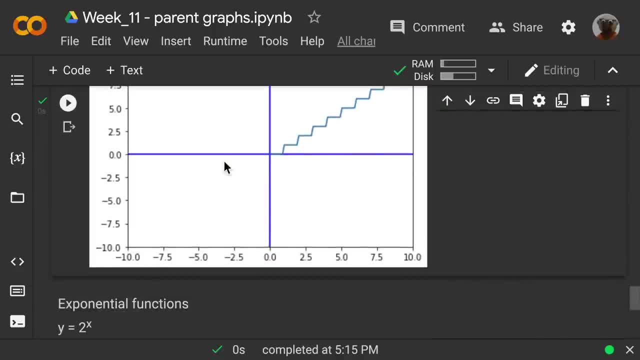 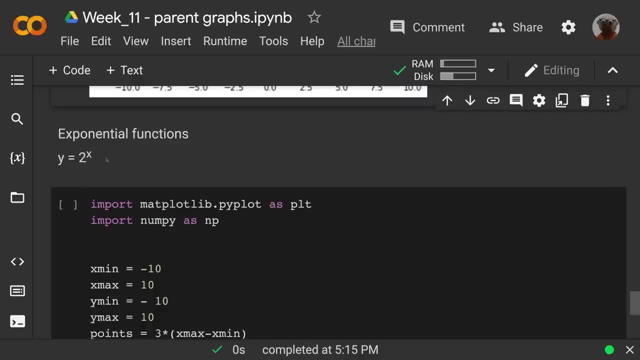 so that's why I wanted to do the loop and show you. so there we go. so that's the floor function, um exponential functions. so now we go from things like x squared to x is the on is the exponent. so what happens when the base doesn't change but then the exponent changes? so 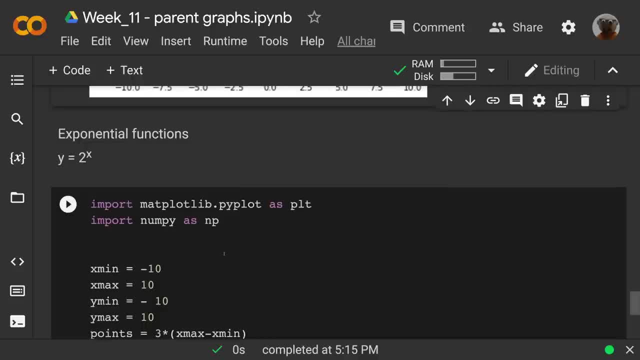 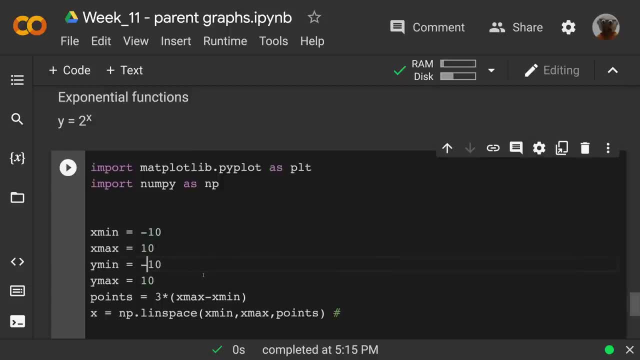 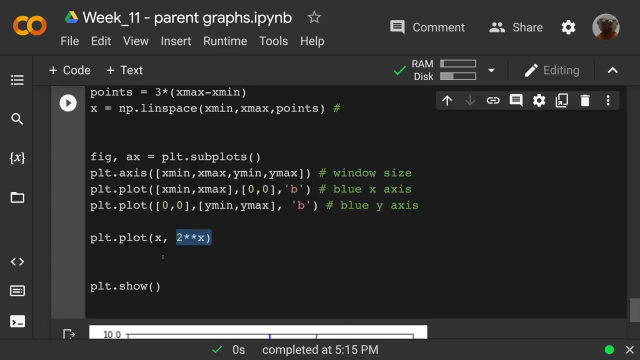 that's 2 to the first, to the second, to the third. well, we can right away see that that value is going to get really big really quickly. and so here to the exponent of x. so we have, we see it gets really big really quickly. and then we 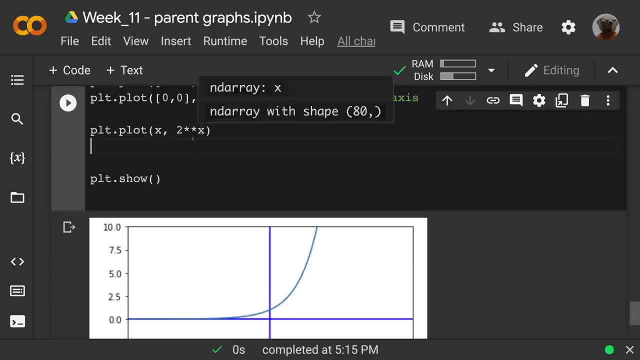 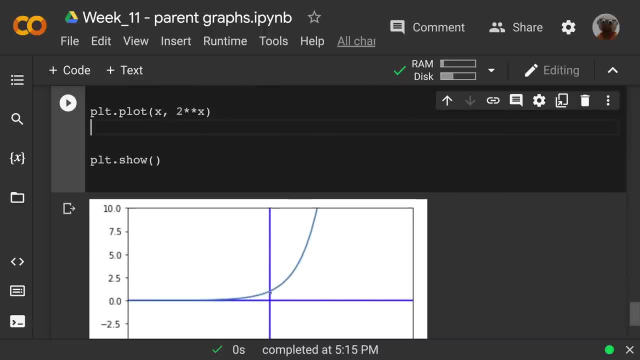 have 0.. and then when we think about our exponent rules, when X is 0, anything to the zero is 1, so all these exponential functions cross the y axis at 0, and then for negative exponents that flips it to the denominator, so 2 to the. 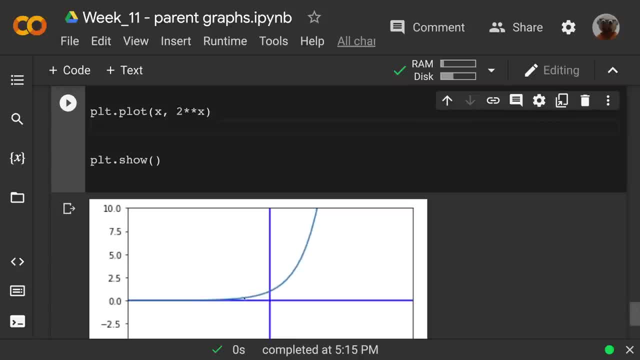 negative. first is 1 half to the negative, second is negative is 1 forth and so the So. it has that curve, but it's not at all a parabola On the left here that just gets smaller and smaller, but actually it will never touch zero. 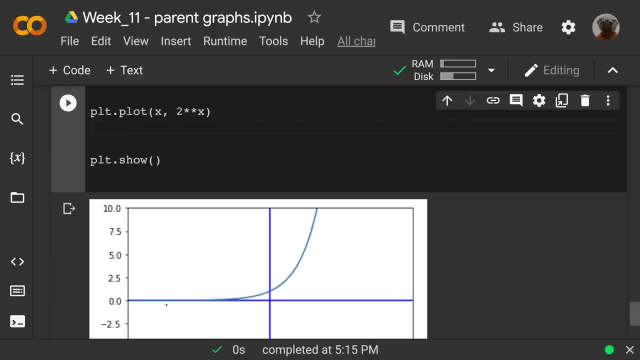 If you get on something where you can keep zooming in, you'll see that it just gets smaller and smaller, but never touches zero. And then over on the right, it just has that upward curve And, as steep as it looks, it actually is never perfectly vertical. 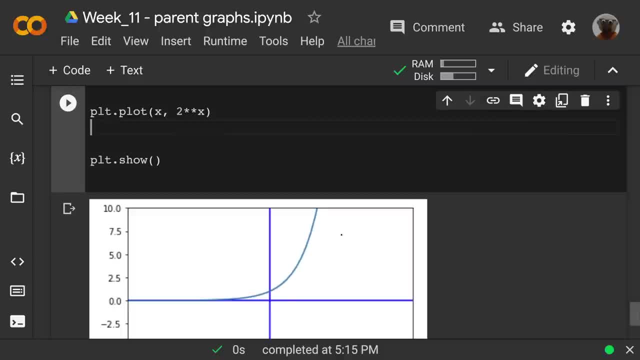 It's just really steep. And so that's the look of all the exponential functions. We use this a lot of times in percent increase, compound interest, things like that. But there we go. That's a lot of the exponential functions here. 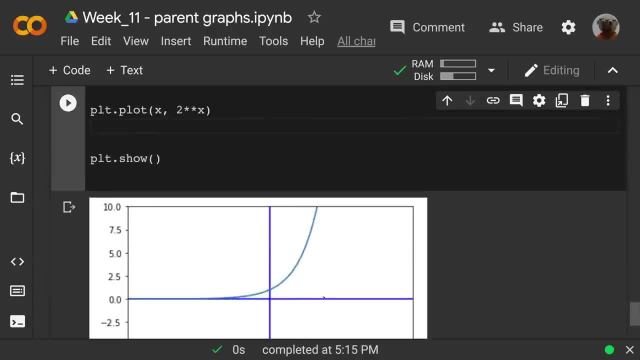 All right, So there we go. So these are all the key parent graphs. All the other graphs you're going to look at in algebra are going to be some version of the exponential function. These graphs- Oh, it's like this graph, but then with some other things that we added. 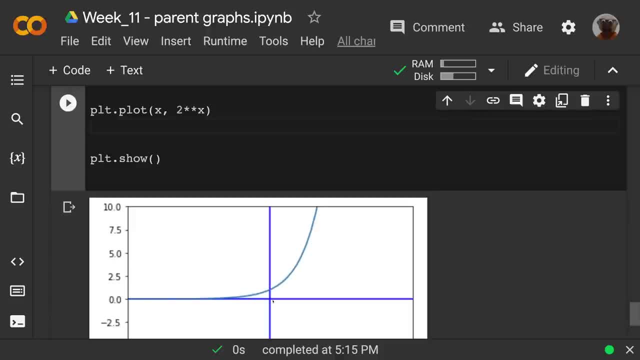 Later on, when we get into another course in trigonometry, the trig graphs are different And one of the big differences is they keep repeating. These are all you know. they do one thing and then that's it. But we'll get to those graphs. 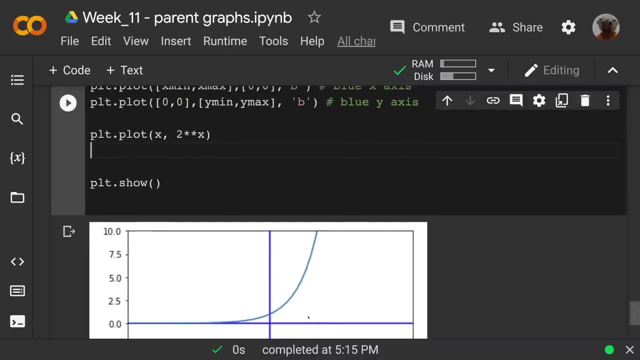 But for anything in algebra, these are all the parent graphs. So when you look at a graph and you want to figure out, well, what could the equation be That generated that graph, You say: well, which parent graph does it look like? 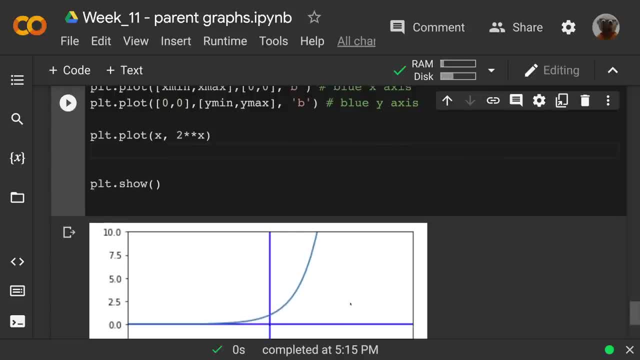 Oh, it looks like this, So it could be, you know, an exponential. Oh, it has that other sort of curve. It could be a different one. So you know. that's why you want to get a sense of the parent graphs. 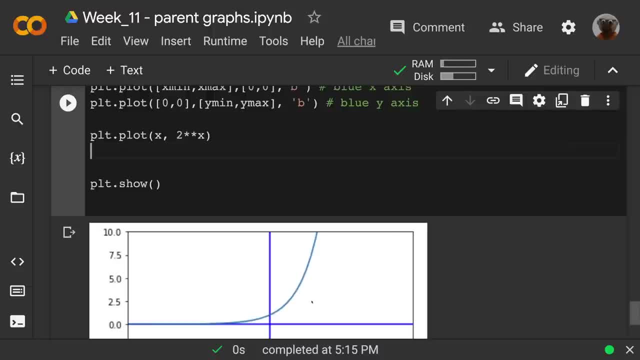 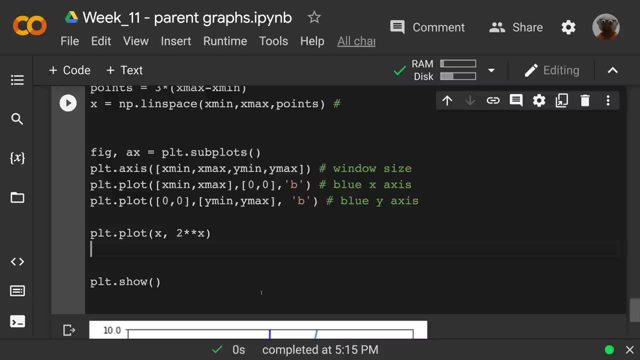 It helps you develop equations to fit different curves later on, And we'll get into some of that stuff. Okay, So there we go, And you will have this as a resource, too, to consult, as you know. take a look. 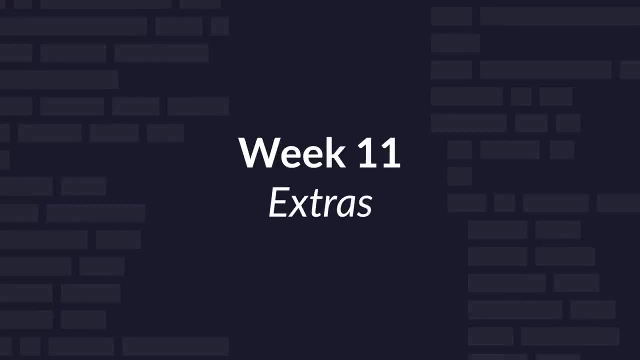 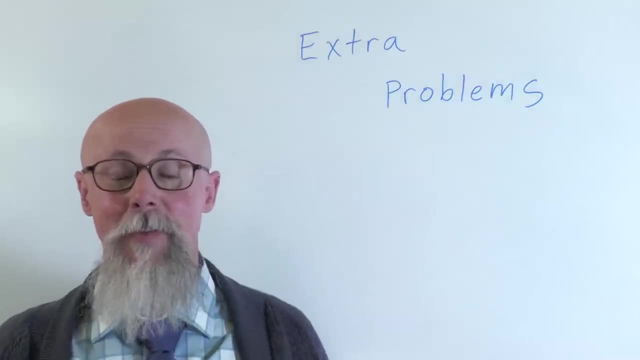 It's the different parent graphs. Now that we've worked through the core skills in this unit, let's look through some extra problems, And I'm going to work through extra problems using the Colab notebook So you can see how you can apply these resources that you're building and use. 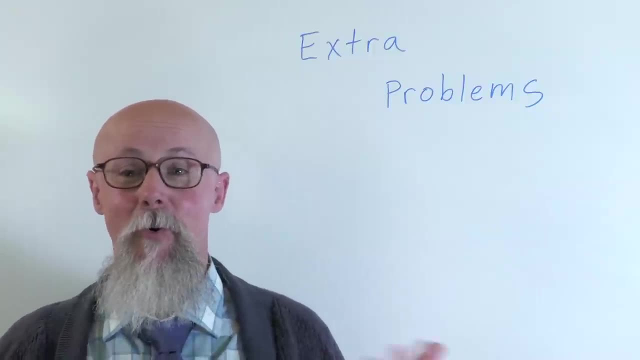 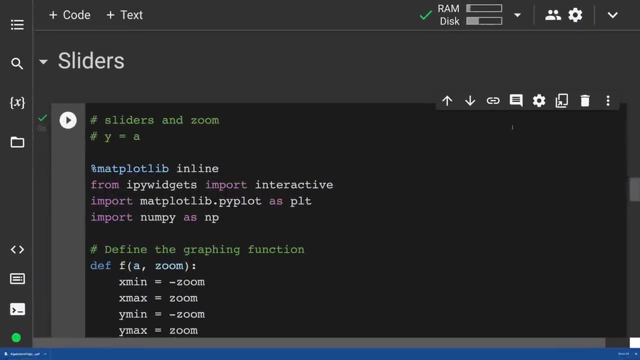 the use these to solve problems that might come up in a textbook or in day-to-day life. So we're going to go through some more extra problems here. So, now that we see these Parent graphs, let's- let's do a little twist here. 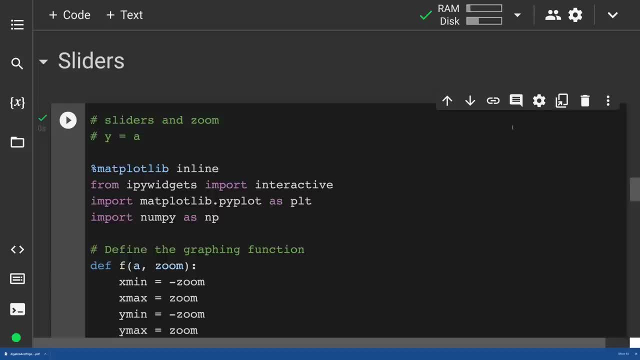 Let's look at the S, these sliders We can add to modify the parent graphs, Cause that's it that they're meant to be modified, So that first one, Y, equals a or any you know value, just it's that horizontal line. 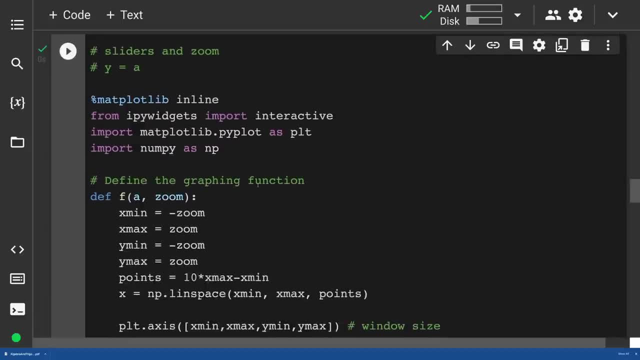 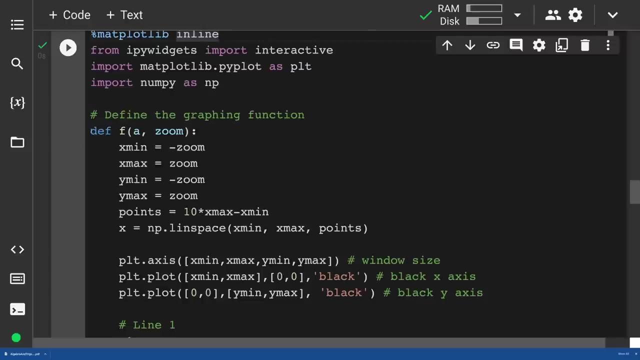 If we add a slider. now notice the setup for the slider that you know we're going to import this inline and it's a widget. So we're going to add a slider and then we're going to add a function to it for the slider, and then all of our graphing is going to be in this function that we redefine here, define and I called it the function F cause I wanted a shorter function, name F of, and then it's going to take a for the slider. 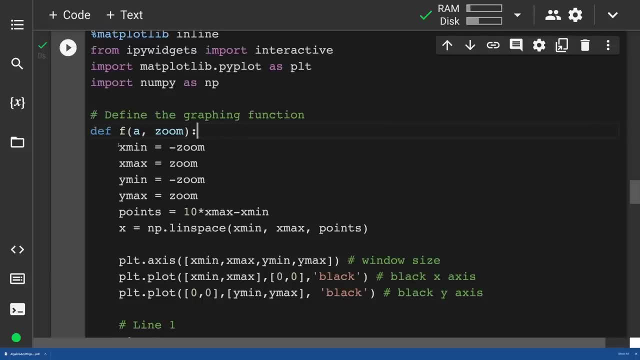 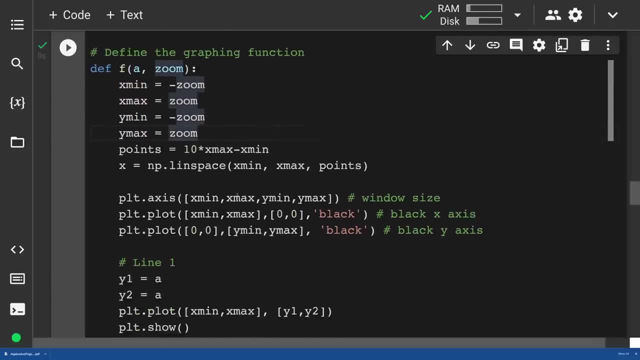 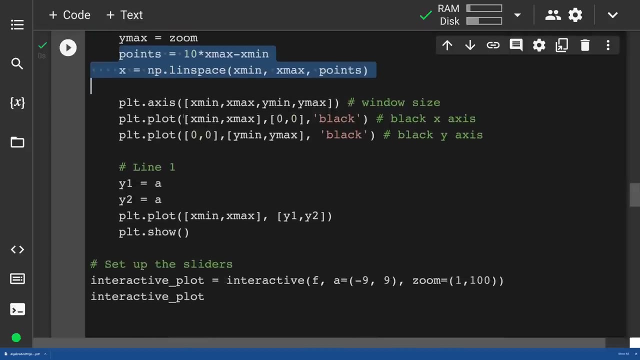 And in this case we're going to also also going to zoom. So all of these values are based on the zoom slider, so you can zoom in and out and we still have these points. But just all the Graphing happens here within the function set the plot and notice all this same thing, but the zoom then would affect all of this. 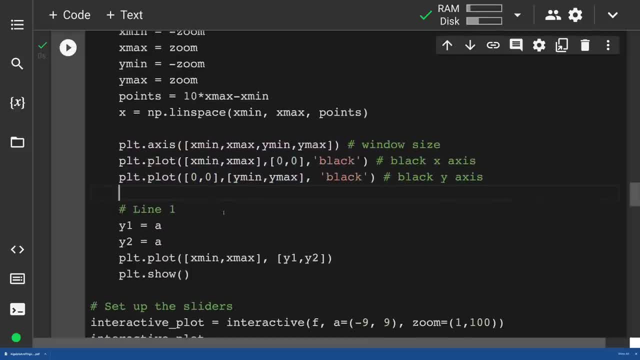 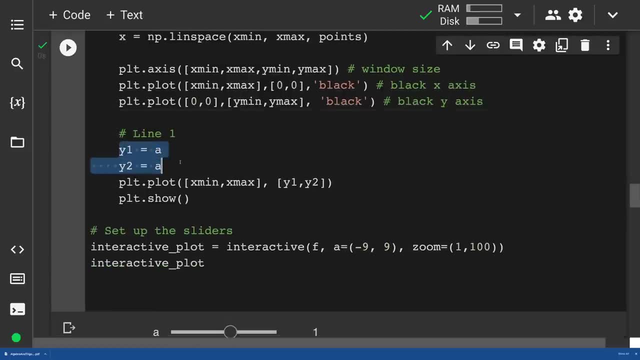 And so, mathematically, you know, if I, if I wasn't writing code, I would just write. you know, Y equals a, but we're going to put it here, I'm going to have two Y values because just this perfectly horizontal line, we kind of have to do it this way. 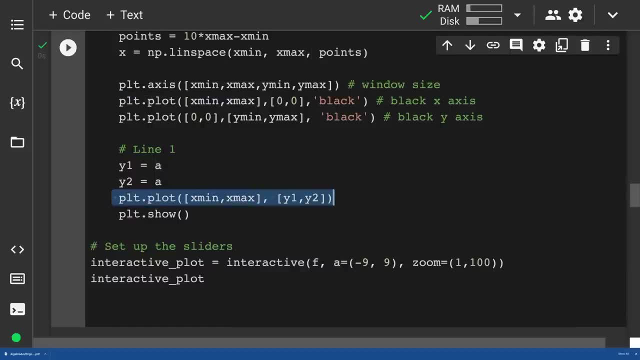 And we're going to plot this Horizontal line, just like we did with each axis, you know, the X values, X min, X max, and then the Y values, Y one and Y two, which are both the same, which is whatever this a value is. 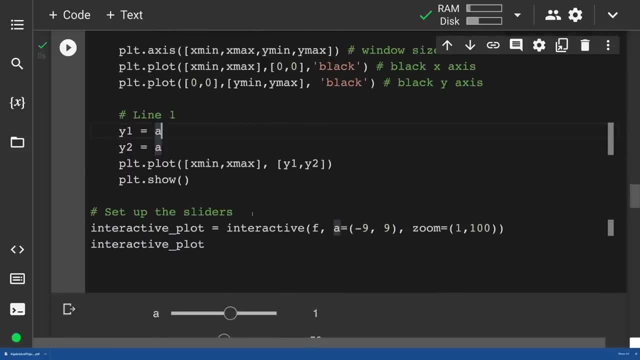 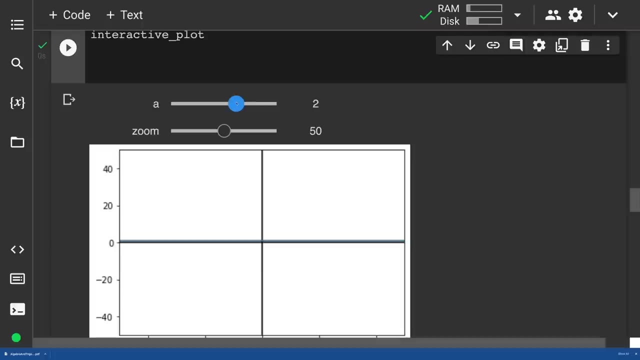 So here's the slider. you know, run this function F a goes from negative nine to nine and then the zoom. So when we run this, so there we go, And as I increase the slider, So we see our general graph and I can zoom in a little bit, but that's what we get. like Y equals some constant. 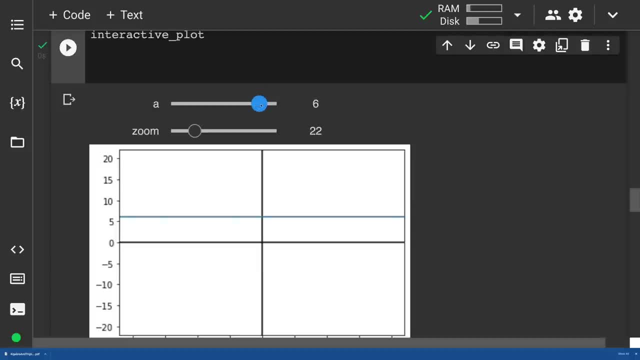 And then I see the slider, that parent graph, it's still the same. look that horizontal line. It's just that, from the parent graph to the child graph, it just, it just changes where it is, See. but then you know the slider, and then the zoom. 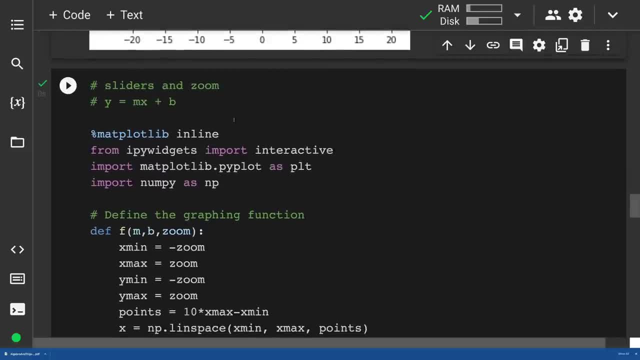 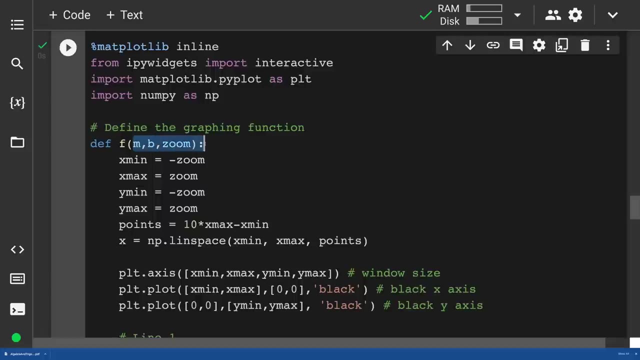 That becomes even more interesting when I have our classic slope intercept form. So now I have Y equals MX plus B. What happens when I use sliders and I'm going to change MB and I'm you know, I like the zoom in there, so I'll just keep that in there. 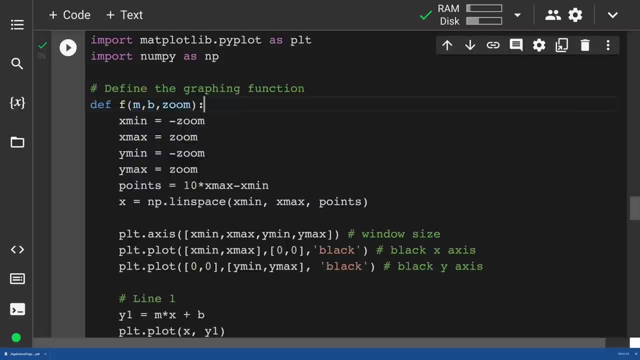 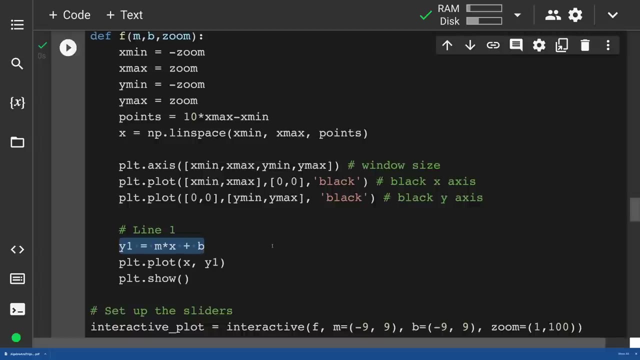 So we have everything for the zoom. now, here and these next few, we can do the normal. you know NumPy, LinSpace, And That's the array that I want to graph for my X values. So here I have: Y equals MX plus B. 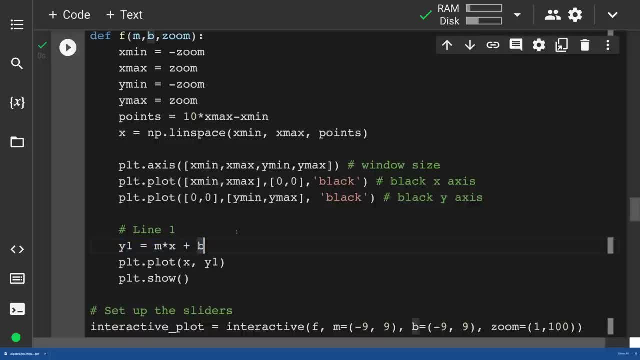 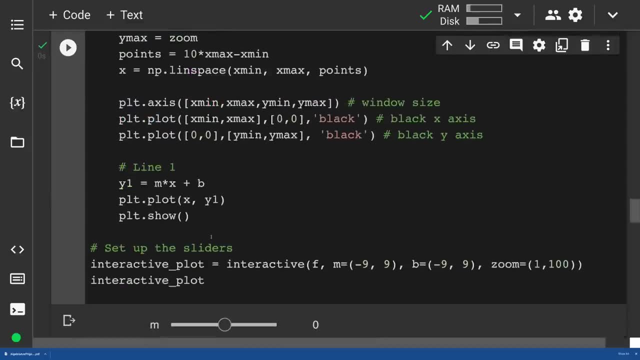 So look at that: M and B are still variables here because that slider is going to affect it And then that function is going to take that input. So now I can have a slider, change the M value, change the B, and I still have the zoom. 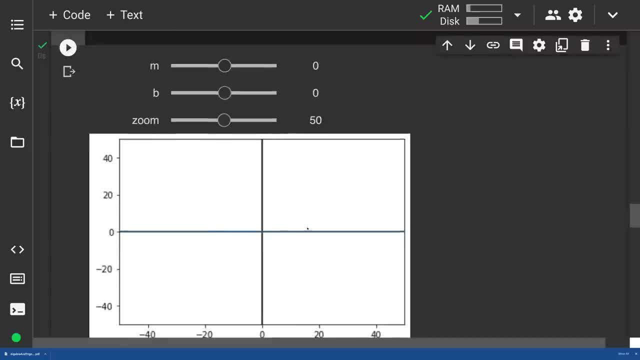 And then this is what I have. So it's right here. Right, Because the slope is zero. But what happens? as soon as I make the slope one? Now I start to see my graph and I can see the slope, And then, as B, increases. 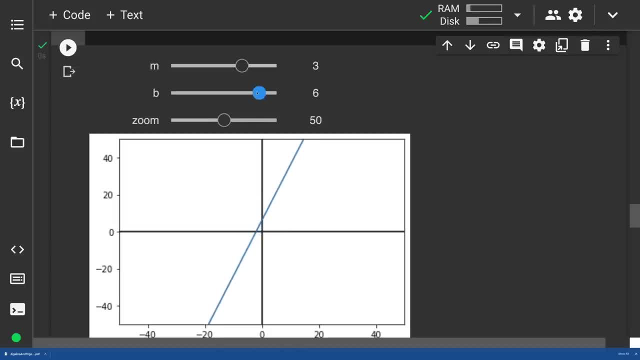 We can see it. the Y intercept moves up and down. There we go, And some of these You know. now we have some more that we can see when we zoom in. There we go, And this particular one. I didn't put the grid on there, but just to show you that, as that parent graph, Y equals X. 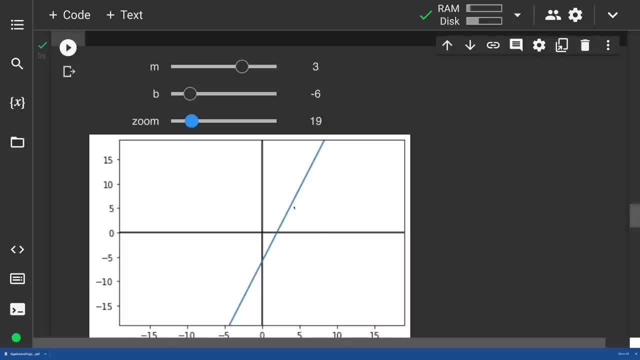 You know, that's really just. that's the paragraph. Y equals X because it does have a slope. but then I can change the slider and see the negative values And from that paragraph. changing these two values makes it its own graph, but it still is that linear equation because that's the parent graph. 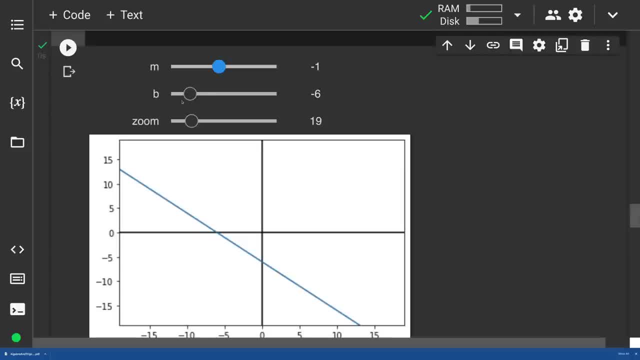 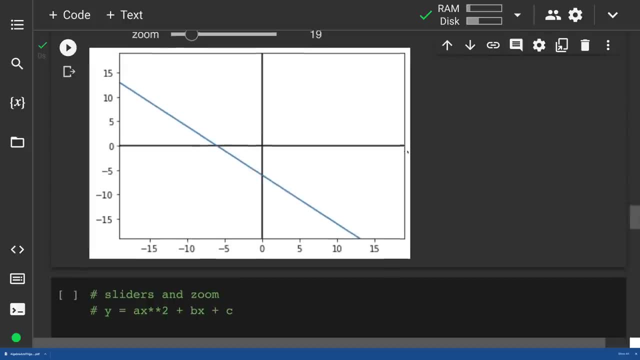 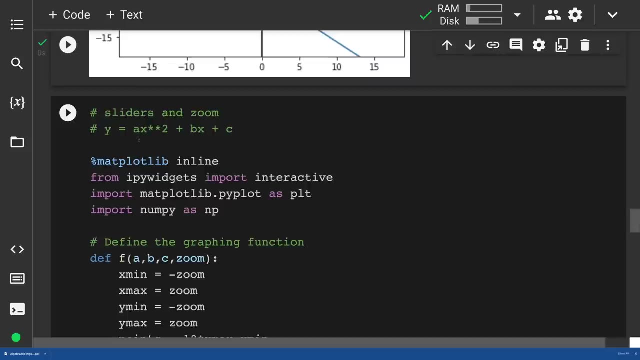 Still is those Core features. But then we modify it a little bit. I can change the slope, I can change where it crosses the X axis, And sliders are a good way to illustrate this. So we have now three variables for our quadratic: AX squared plus BX plus C. 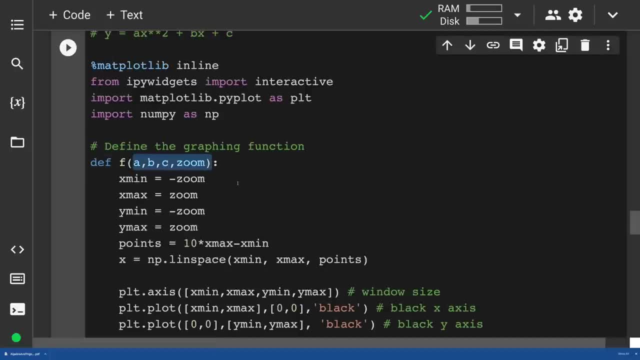 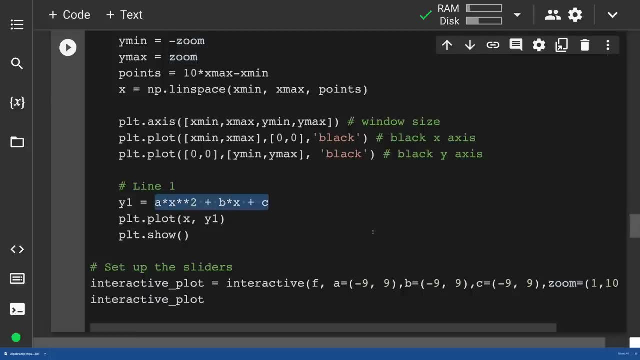 And so my function. I'll take A, B and C and zoom in. So then my Y value is just this standard quadratic. I remember X squared is the parent graph. You know, A is one and then just X squared. That would be the parent graph. 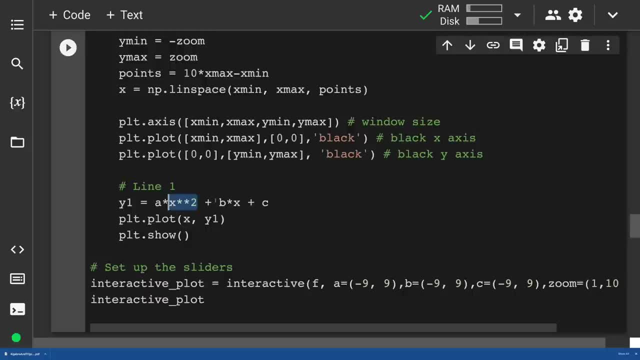 The simplest quadratic, It's a parabola. But then when I have these three, it still has that core feature of the paragraph. It's still a parabola. But then I change and we can see what A, B and C. 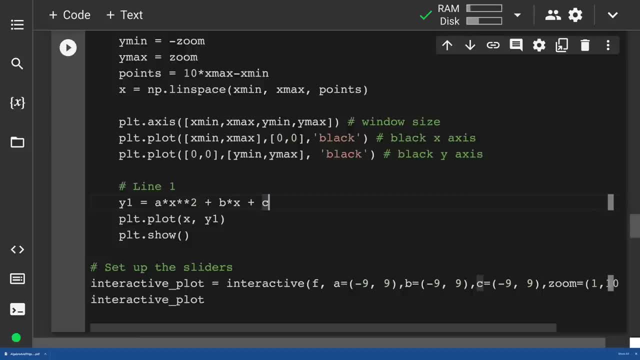 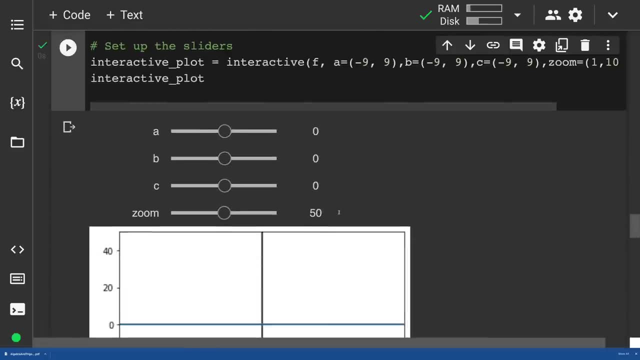 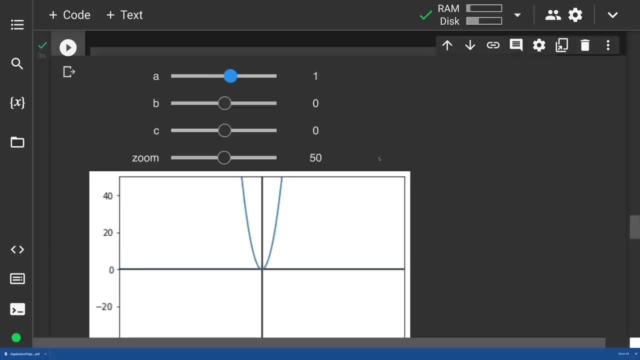 do to these, so we have this interactive. i'm going to adjust a, b and c and as well as the zoom, and so we see it defaults to right in the middle, so let's just put a. now that's one, but we can use these slides to see what does. what happens to the graph when 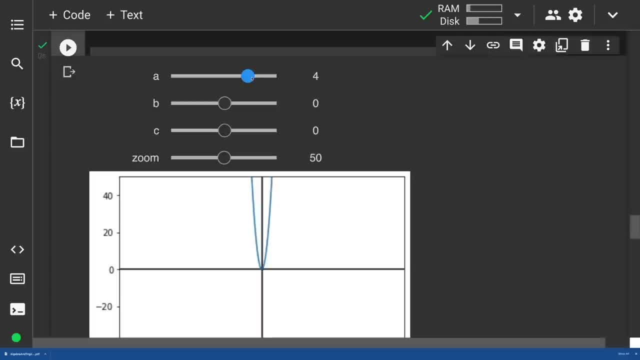 a increases. you see it gets narrower. and then what happens? zero, it's not a parabola anymore, but then, as it's negative, it flips it down. there we go, so we can see how these affect. you know, we'll bring it back up to positive like a smile, then we can take a look at: well, i'll jump. 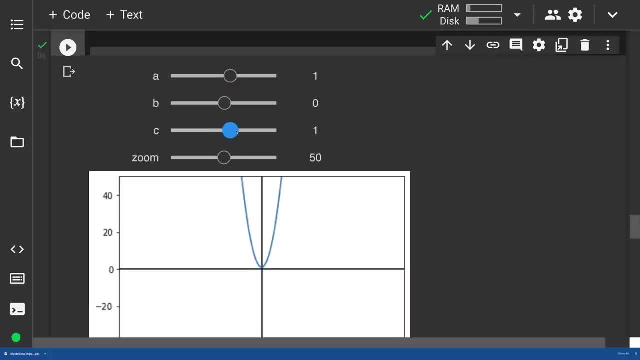 to c next, because that's the easiest. it just same shape, it just moves it up. or if c became negative, same shape and it moves it down. and see, each time i move this the, it runs the function again and then recalibrates it with these new values. 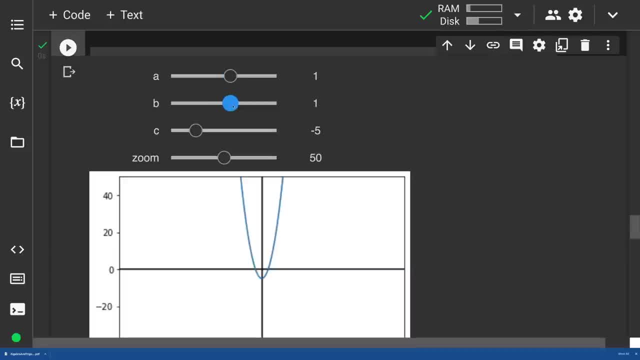 and then b. i think is one of the most interesting- because i move it, as b increases it dips down to the left, kind of interesting- and then i can bring it back, and then as b decreases, it dips down to the right. so just some interesting things that you know. so this would be a, b and c, so this would be x squared. 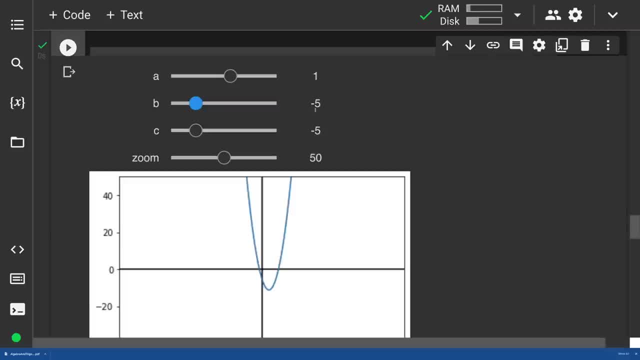 minus 5x minus 5. that'd be the equation here. or then x squared minus 5x minus 6, and we're going to do a little bit of a re-evaluation here, and then we're going to do a little bit of a re-evaluation. 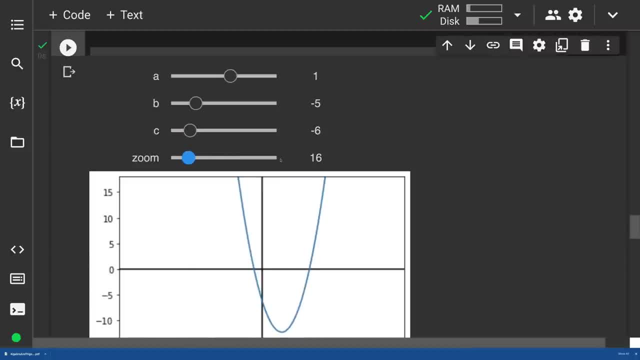 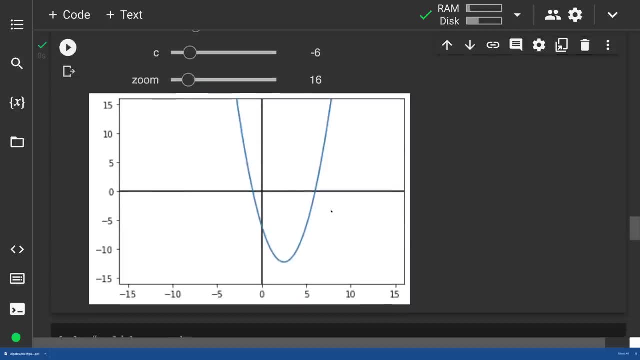 We can zoom in and see. you know, I didn't put the values on here so exactly, but you could always do that too. So we see these sliders Now the reason why I like this and I want you to notice with absolute value how similar 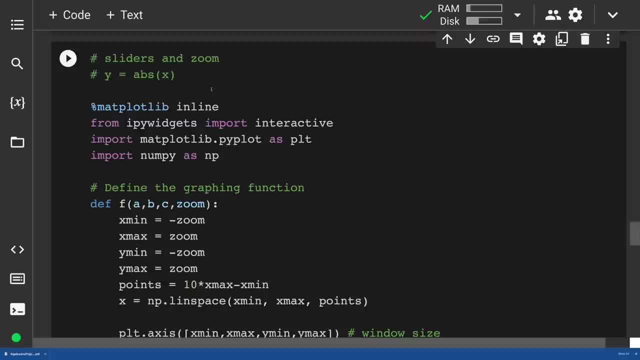 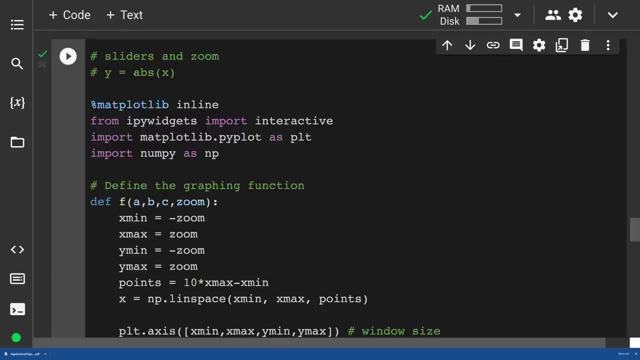 those patterns are to the x squared, the absolute value, Because, remember, whatever x is, if you square it it's positive. Absolute value also then just makes it positive, But the core absolute value function. so you see absolute value, but I'm taking in three. 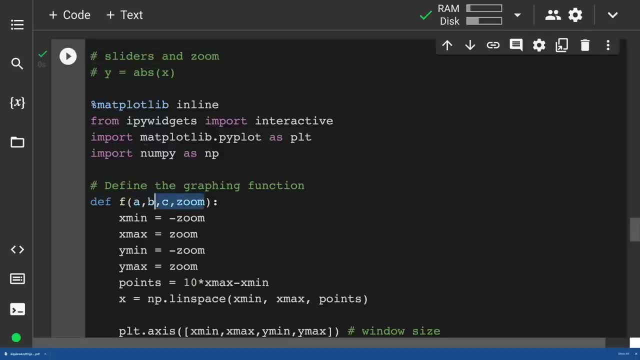 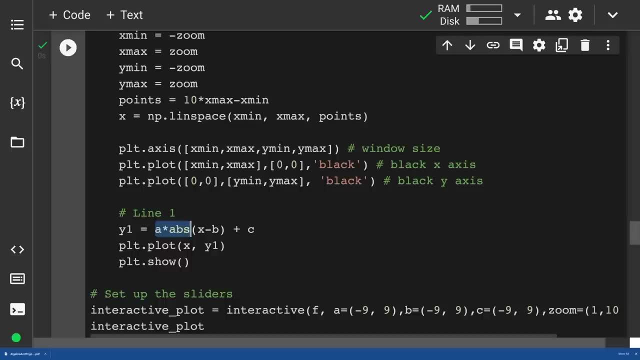 different values here from my absolute value parent graph. I still have three sliders. Why? Because I have a times the absolute value And then inside the absolute value I could have x minus b. that's where the b shows up and that shifts it left or right. 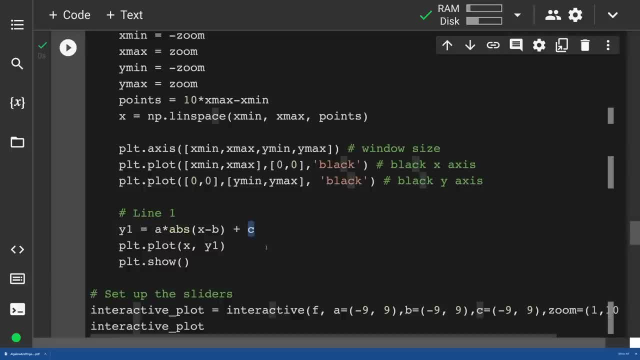 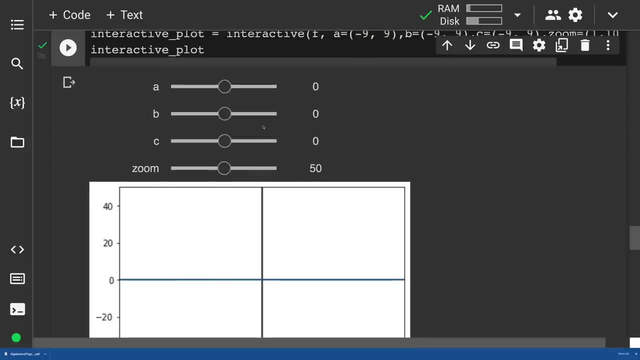 And then plus c shifts it up or down. So we see that plus c shifting it up or down, And let's take a look at these. So again, a is zero. I've got nothing. soon as I change it Now, I have my absolute value. 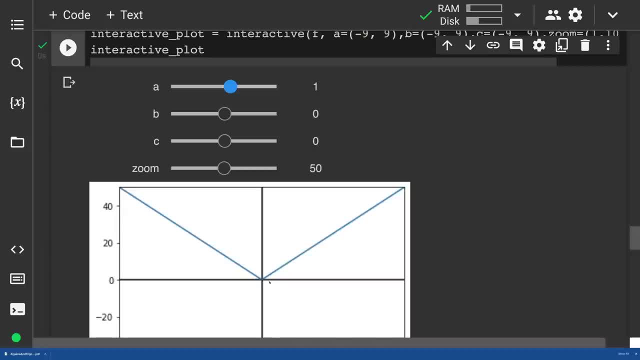 And of course the big difference is: this is linear, each line is linear, but then it comes to a point Because, again, positive x values were negative. the absolute value makes it positive. So we see some of those similar patterns, though as a increases a times the absolute. 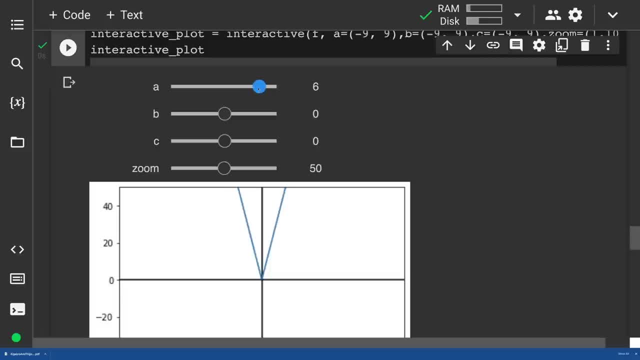 value. this gets narrower, just like it did with the parabola, And c keeps the same shape, but just moves it directly up Or Moves it down. And we have b. this just moves it exactly side to side. So that's you know. this is where, unlike the parabola, there's no other deeper curve. 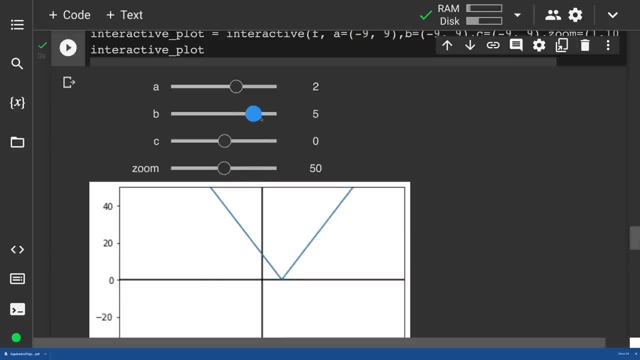 to it. It just moves it exactly side to side. So there we go. Okay, There we go. And even if c- you know c was more- it still, it still moves it side to side. So b is negative eight. 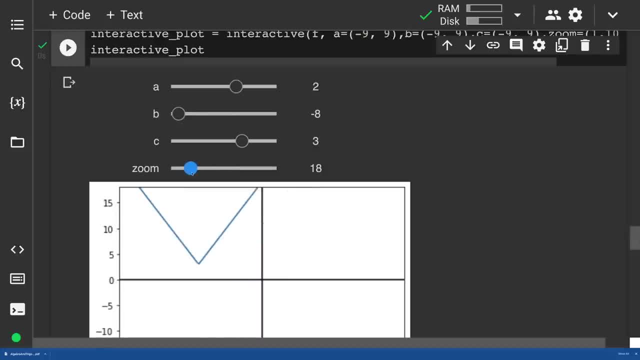 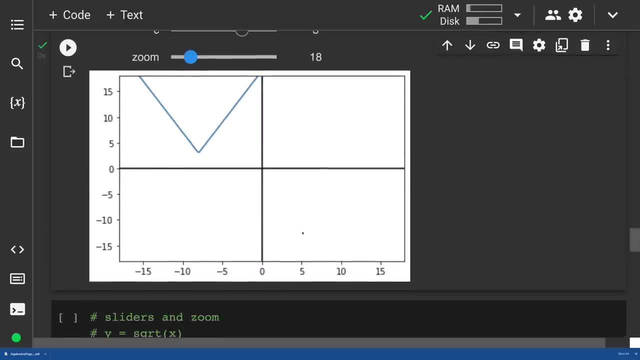 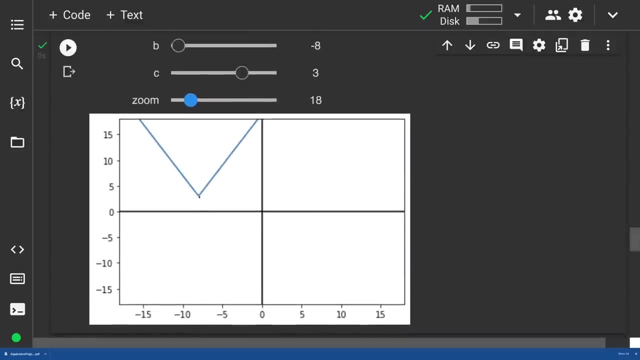 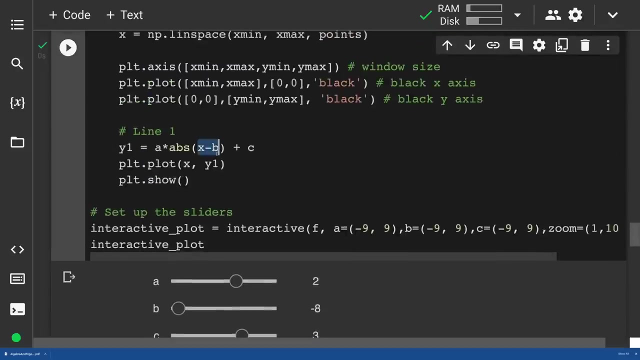 So the, if we see the zoom here, So if b was negative eight And we see that that is the x value, So it's at negative eight, And then, because it's b, it's x minus b is the is the formula. 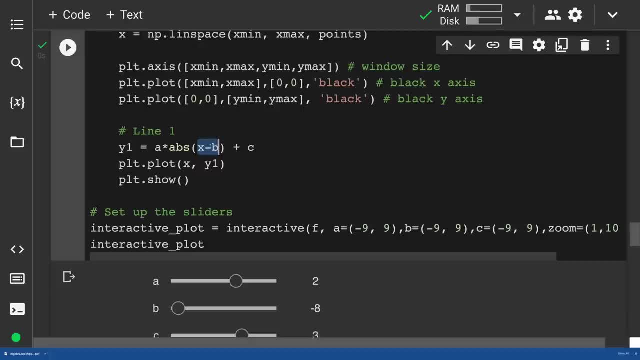 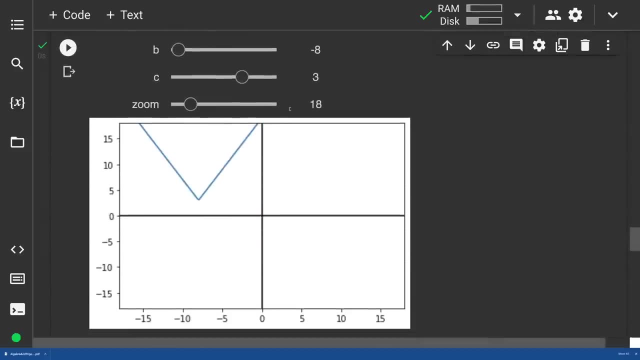 So if b is negative eight, then that means that's x plus b. negative negative makes it a positive, That's x plus b in the inside, the absolute value. So So negative eight and then c is three, then we go up three. 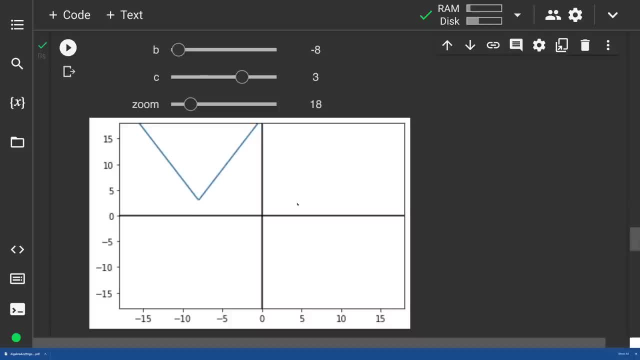 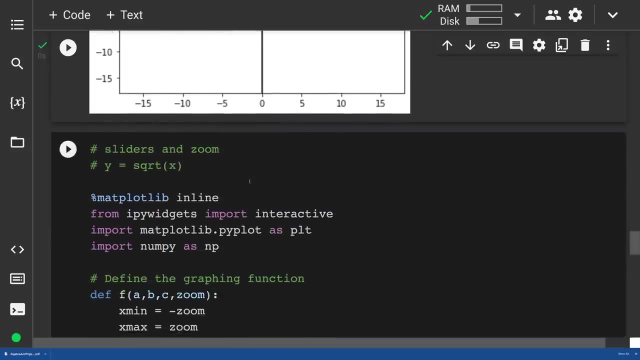 So we can see again- you know where is that point- And we see the basic absolute value and then what each of these things do and how. it's very similar to the quadratic, but that has its own, its own things And we can do this. you know, those are the most useful, I feel like, for a lot of algebra. 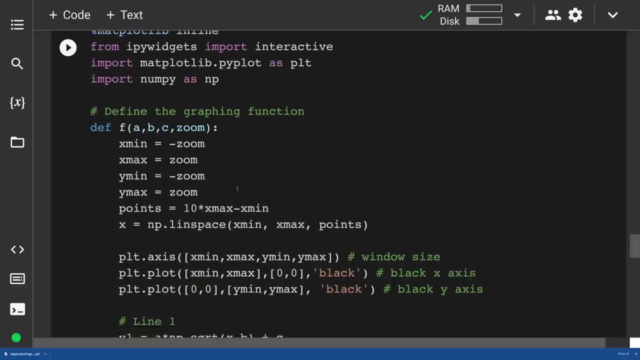 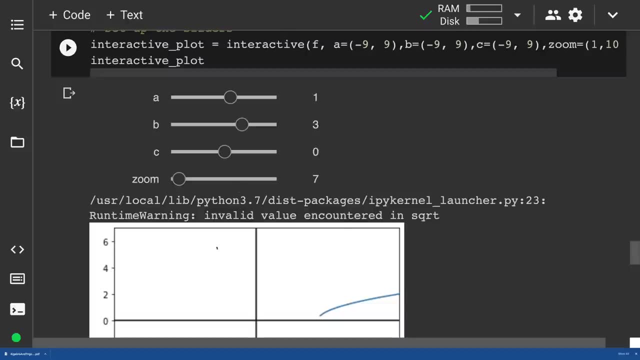 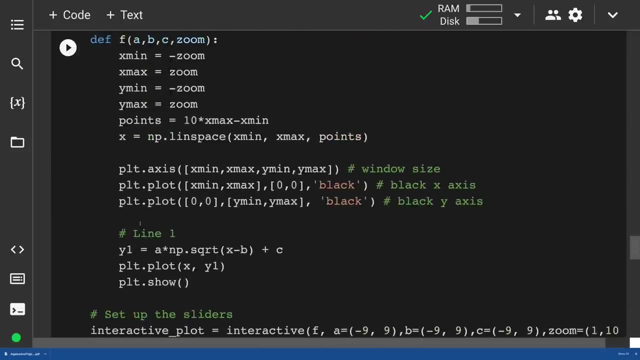 you know, more commonly useful. But square root functions can have an advantage. You can have an slider too, And this one, um, it gives a runtime warning, which I just left in there and it still ran, because the you can't take the square root of a negative number. 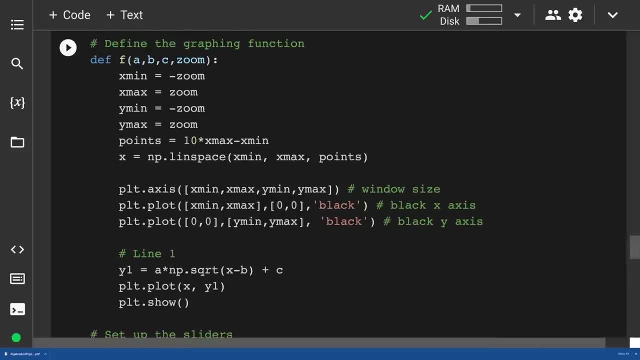 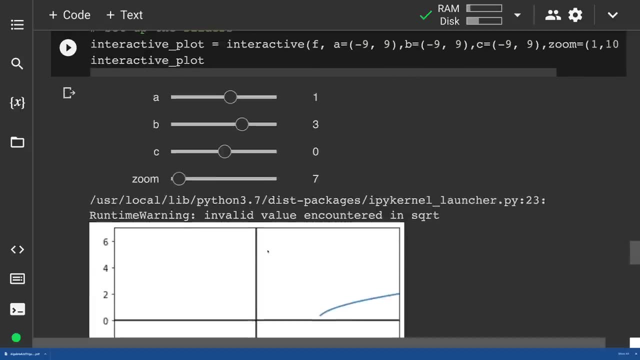 So you know, I still have all of these different zoom values that I could. you know, at some point I get a negative number and it just does not compute, it won't show up, but it actually. that doesn't break this. 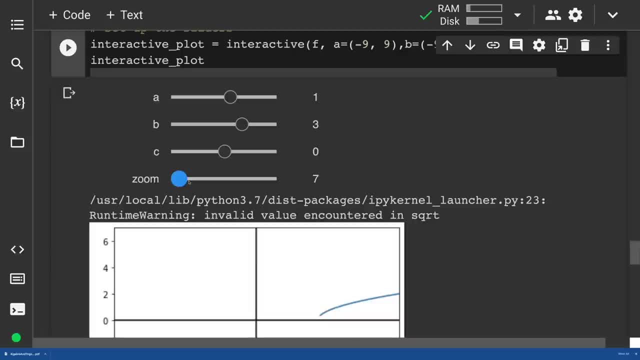 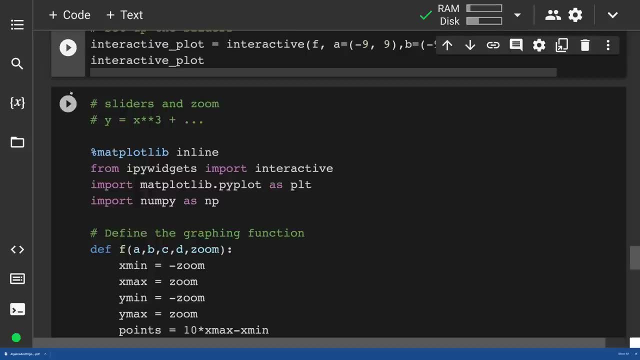 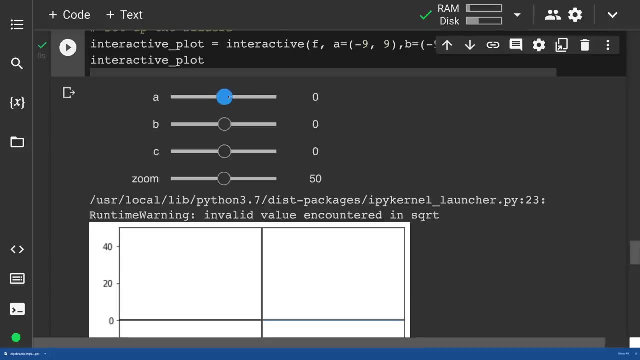 It will give me the error, but then that's it. So here, if I take a look at B and I make B zero here if we run this again, so again everything zeroes out. where is it? But if a is anything, there we go. 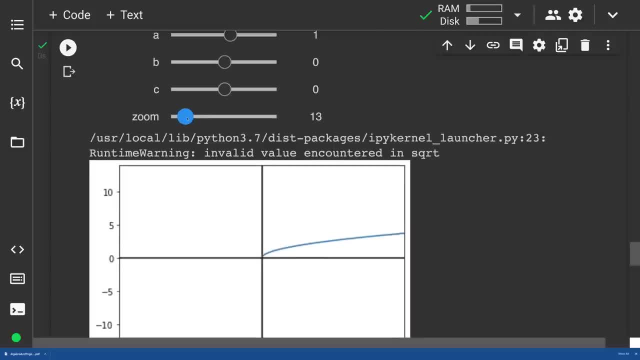 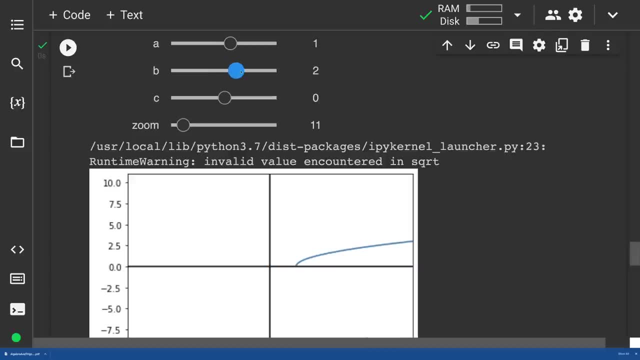 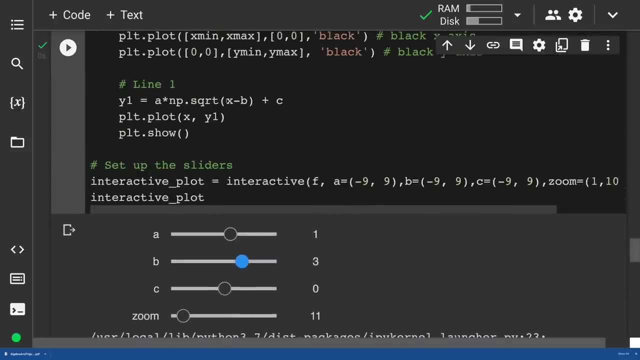 And we can zoom in a little bit, see this curve a little bit better. There we go. So, if a is anything, And then we can zoom in a little bit, And then we see B, it moves it. But remember it's because, like the other ones, X minus B is the formula. 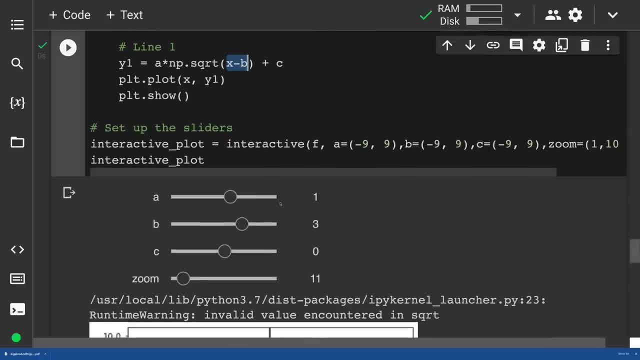 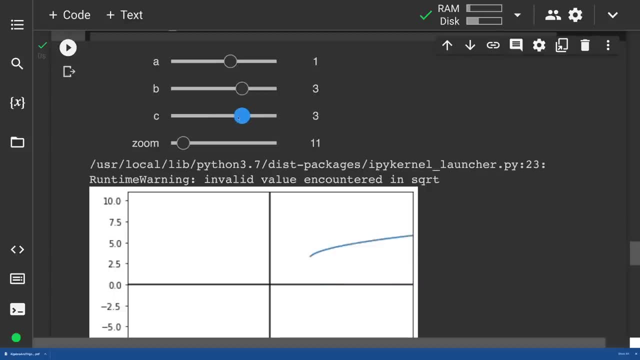 So when B increases, that's really X minus three- moves it three to the right, And then C also, you know, moves it up. And again we're looking at that point where this starts: Yeah, That square root function starts. 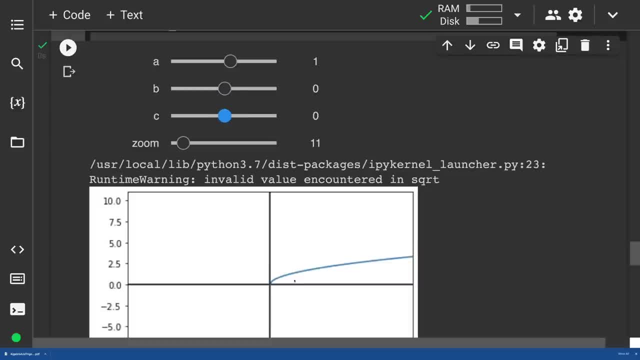 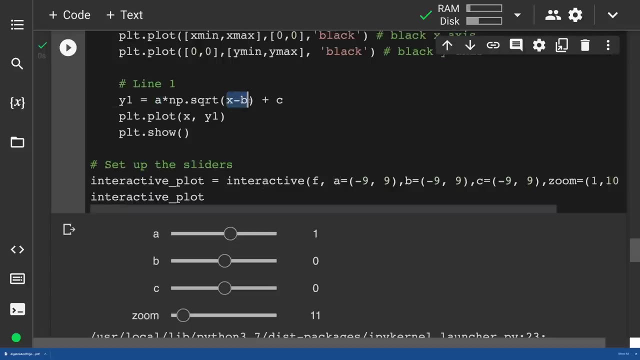 Whereas if B was zero and C was zero. you see, that's where we start at the origin: zero, zero. So we see, you know your basic square root graph And again you have these different values. You can have a times the square root and then square root of what X minus B, And then I 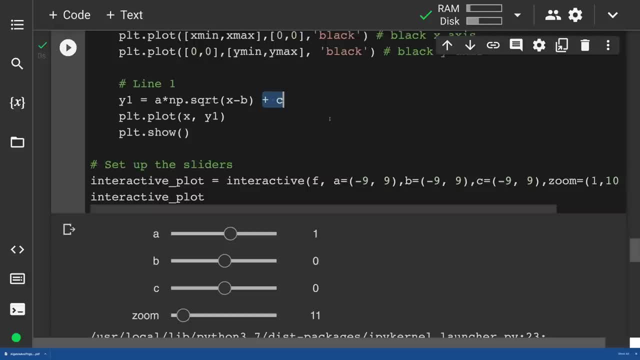 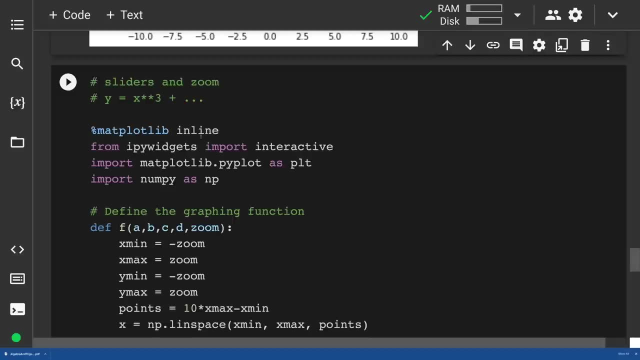 still have plus C outside that can shift it up or down. So we see from the basic parent graphs All these key things And we start- hopefully you're starting- to see the patterns of how this comes up and you can have these sliders with all different. 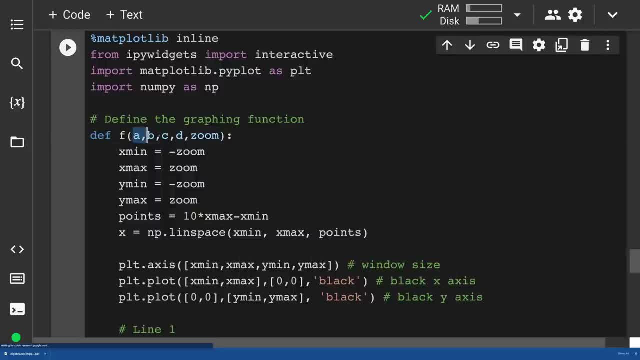 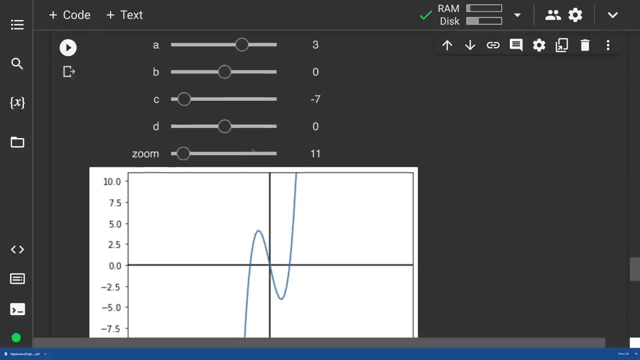 So if we have X to the third now, four sliders and we can see, you know, X to the third, Now for this one. I just left it as this to show. this is what happens. you know, a increases this. 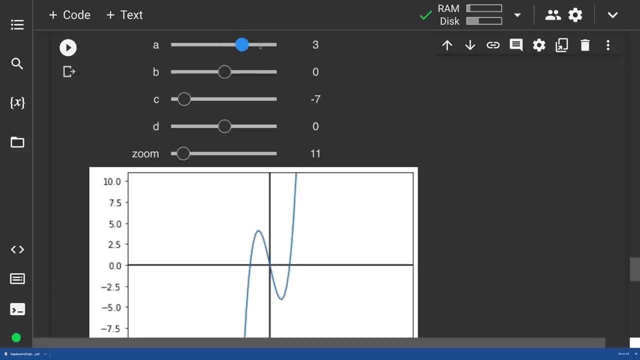 Yeah, You know you can make it a little bit narrower. but B is even zero, C is negative, D is even zero, crosses zero, zero. But I just set up, you know that's where you get. you know some deeper dips in your 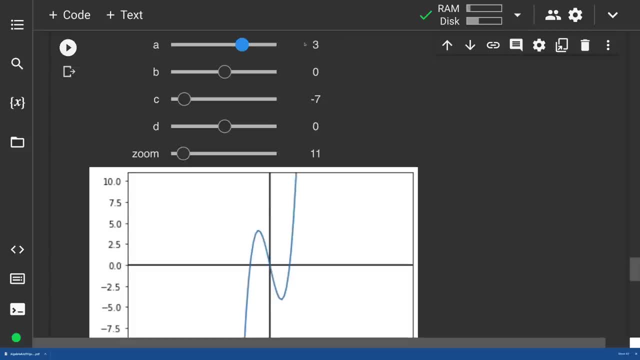 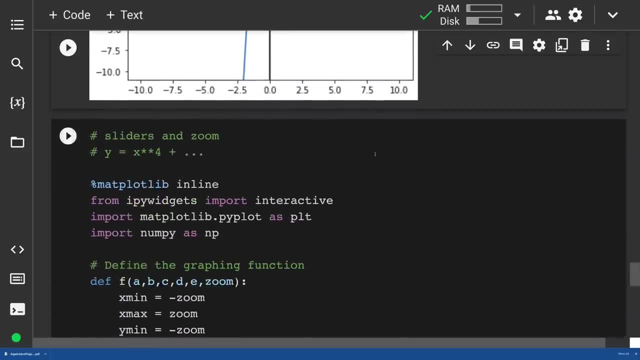 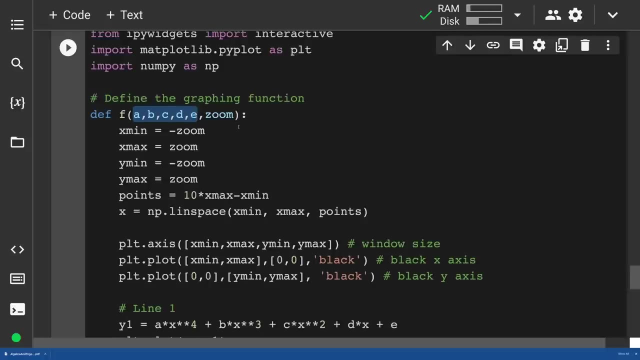 X to the third functions here, So, and it's usually some mix of positive and negative coefficients that give you these deeper dips And you can do the same thing, X to the fourth, And you can have five sliders, because X to the fourth would also have a times X to the 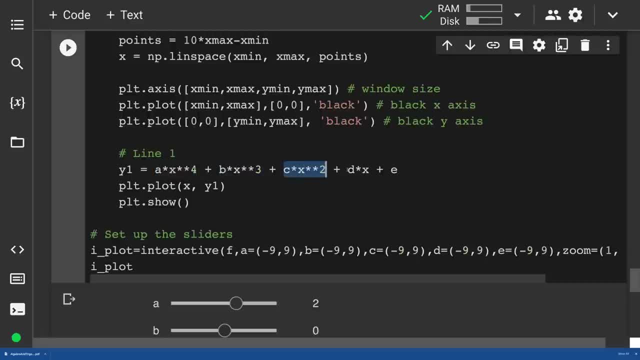 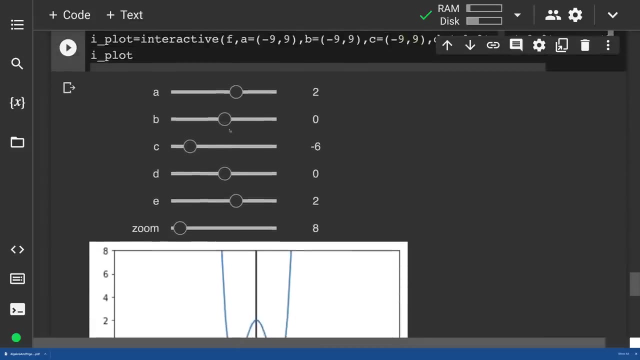 fourth, And then B times X to the third, C times X squared D times X to the first, And then the constant E, which actually would be times X to the zero. So there we go, And having these, you know, we can adjust these. 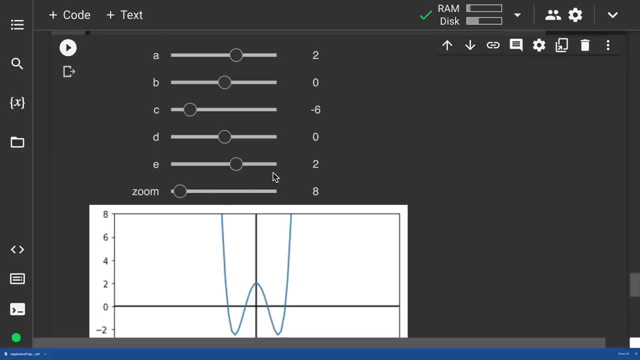 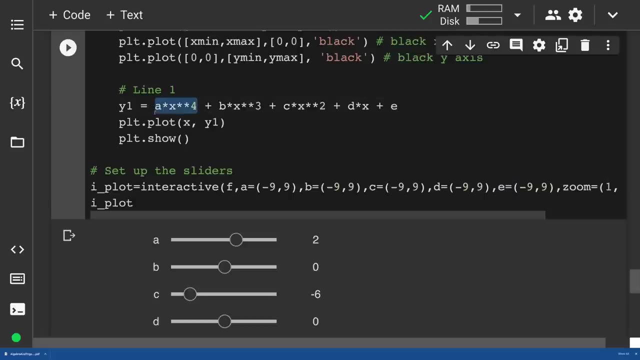 They're not going to be the same. They're not going to be the same. They're not X. These are not always symmetrical, but I picked one that actually could make it symmetrical, And what that is is notice where the zeros are, because X to the fourth, A is the coefficient. 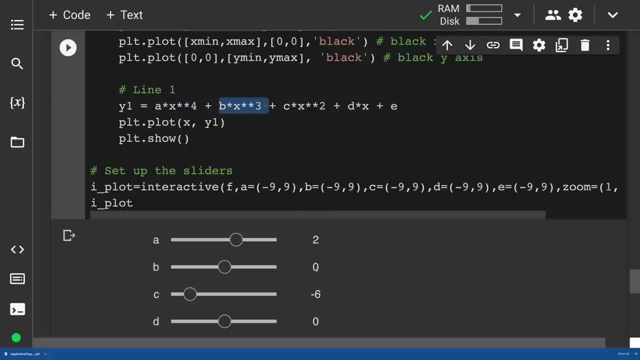 I made that two. X to the third. B is the coefficient. I made that zero. X squared, C is the coefficient negative six, And then X to the first. I mean that zero. it's symmetrical because all of the even exponents have coefficients. 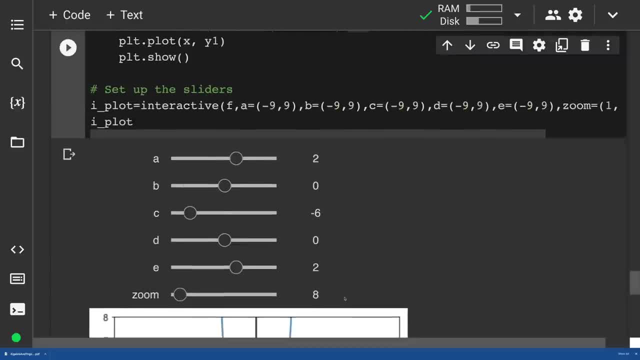 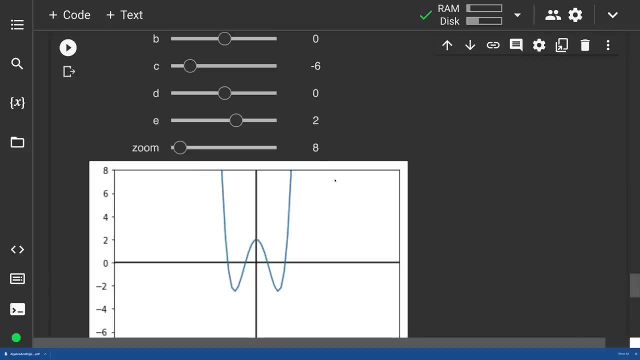 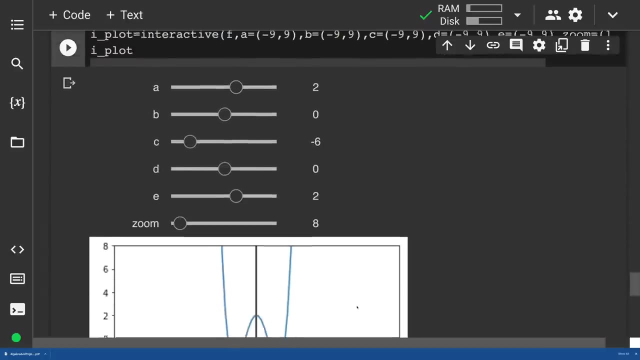 and the odd exponents zero out. So these even functions happen only if I have all even exponents. And notice I can have an E value because E is X to the zero and we'll count that as even. So there we go. So. 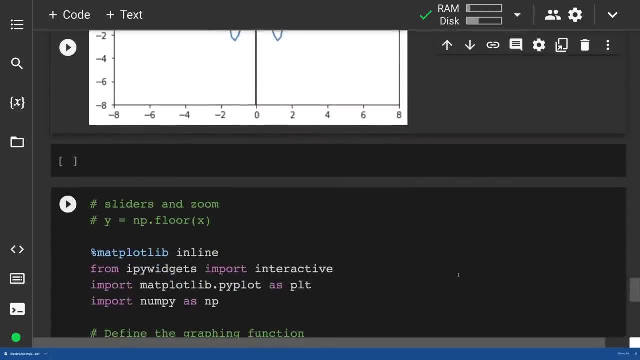 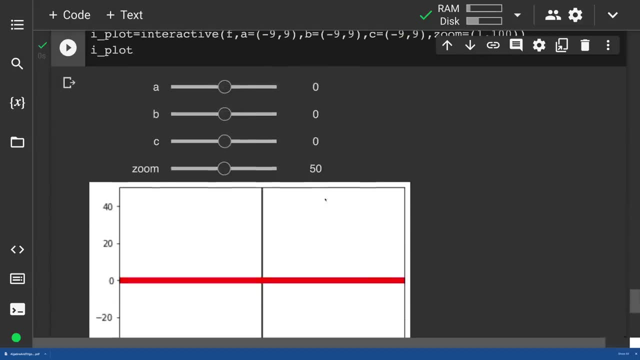 So some things you can see when we have sliders. you know, same thing with this floor function. This is just kind of cool, And so what I did here is I, you know, still with the zoom, but I made this floor function. 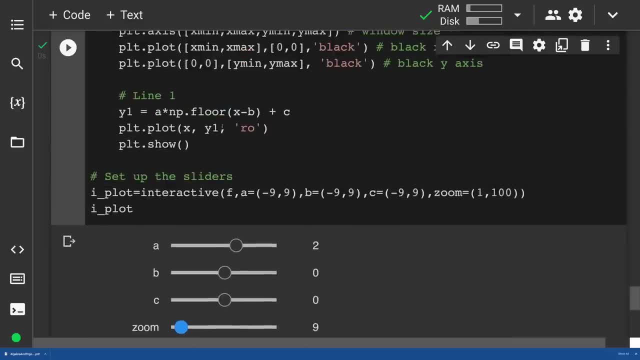 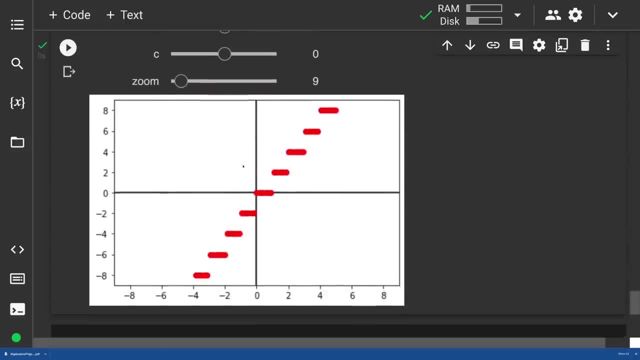 I did this, um, to make these a bunch of dots, Okay. Okay, Displays the fourth floor function. That's really like. this is really the floor function And I made these dots. you know to plot the points instead of lines and you know the. 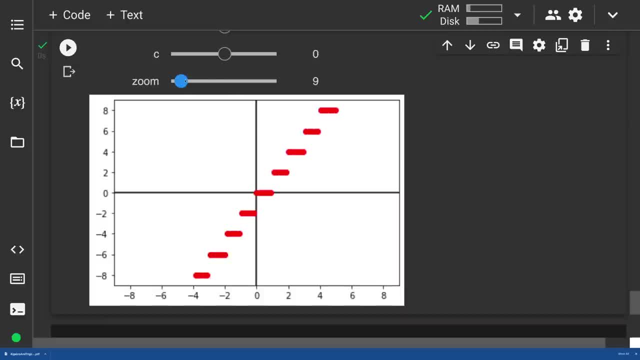 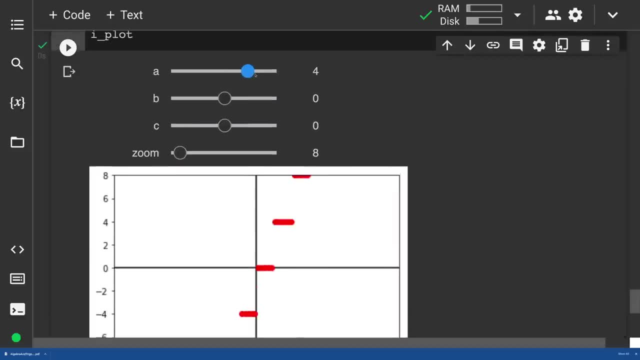 big enough that they connect so you don't see spaces between. but that's really. this is really the floor function as we, as we know it, And we see that. you know, if a increases, it just gets steeper and it could be negative. 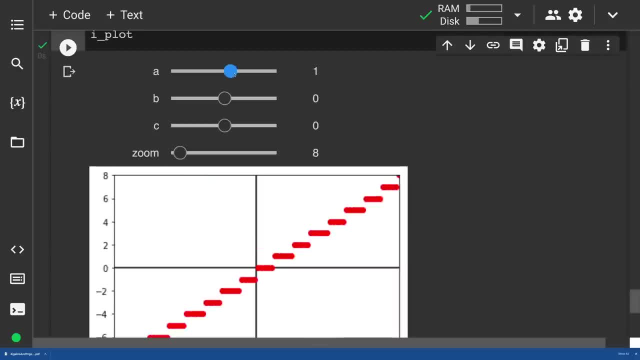 and it could be like that, but still has that step. look to it so and then see it's almost- yeah, i guess it's noticeable, there you go, but that's it. so this is the floor function. we have the different steps and you see, we still can have that's the parent function, just the floor function, but then and the floor. 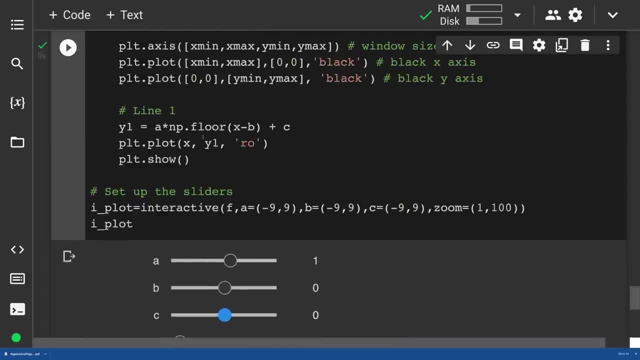 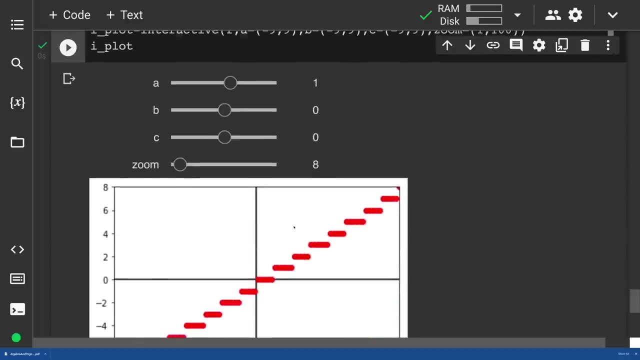 the general parent function would be: yes, i would have a times this, so i keep that as one, and then you know nothing else going on. that would be the parent function, and then we can adjust things. so all these, you know that, taking it beyond the parent functions, you can have sliders. 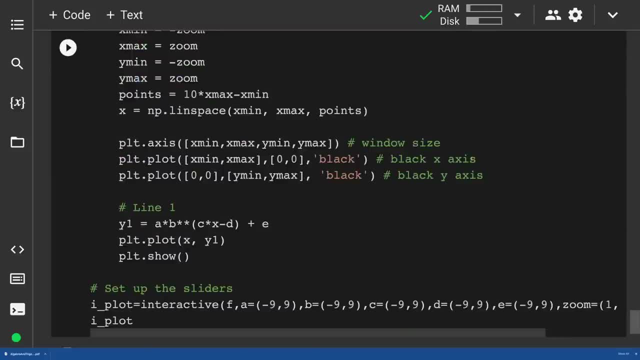 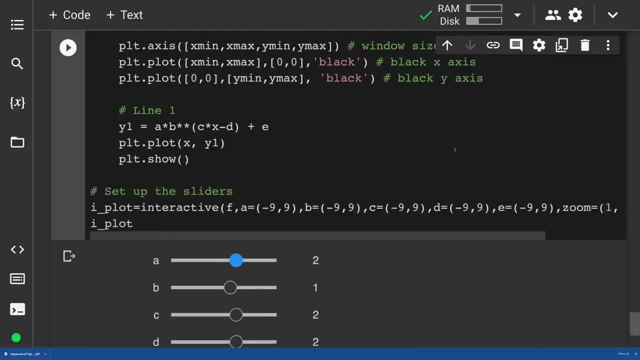 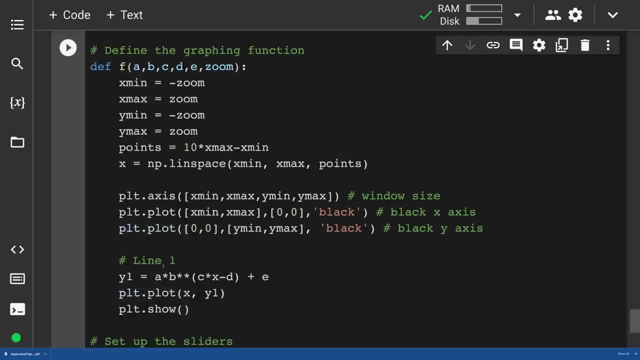 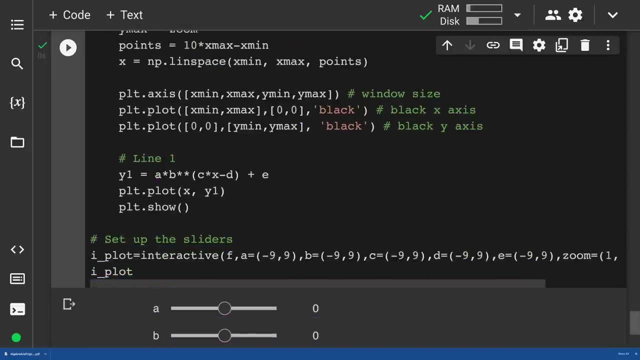 and you know all kinds of other things for, um, you know, there we go. some, some other functions we can have all right. um, oh, this was the uh exponential function. we'll end it on this here, that if i have this, so i still have my a coefficient and then b to the exponent of something, cx minus d. now, 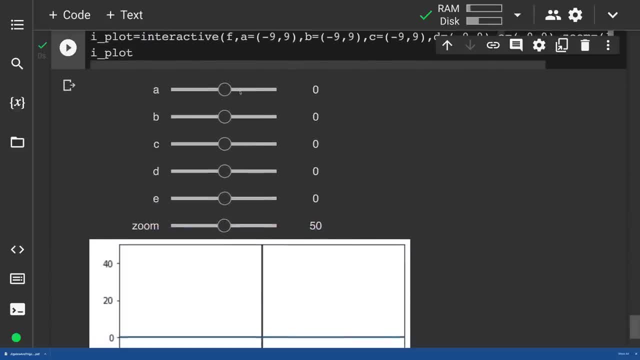 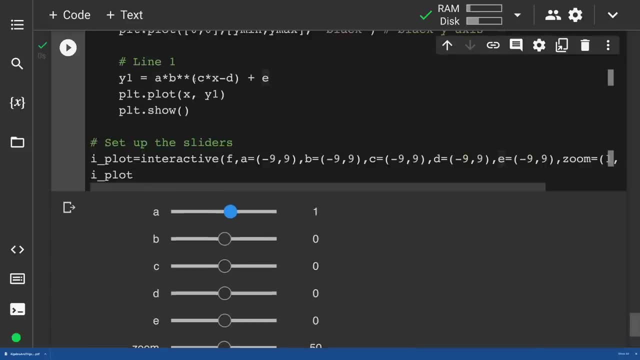 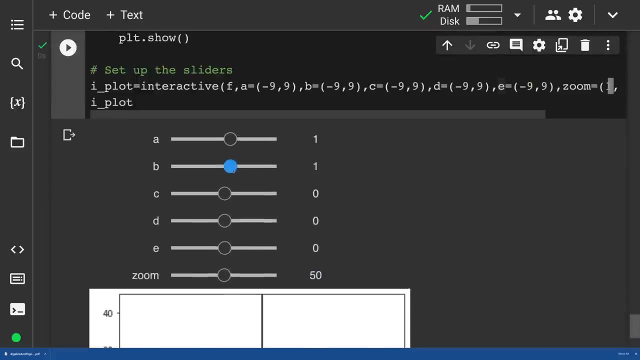 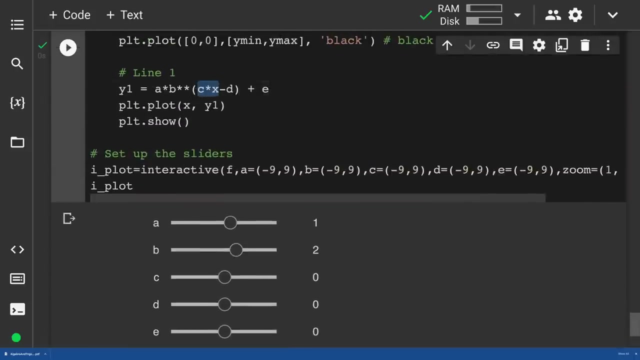 nothing going on because a is zero. but if a is at least one, but still nothing going on, because i have uh, b has to be a value and it has to be one won't do it. it has to be greater than one. and then c, it's c times x. this won't do it because that would make the exponent zero out. so again, 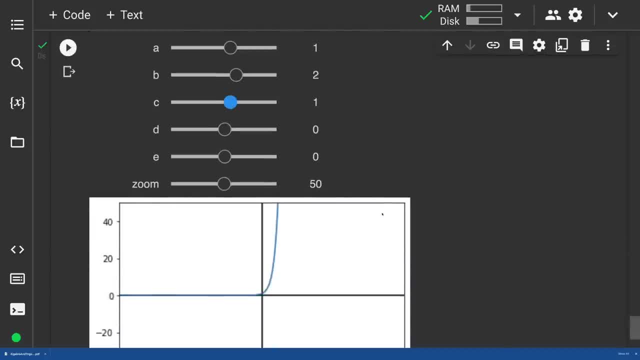 it would be a constant. that has to be at least something, and it's there we go. we can zoom in a little bit. there we go, and you know, d that could shift it and e that could shift it up, just like we were doing before. but you see these- there's a few of these- that needed to be non-zero. 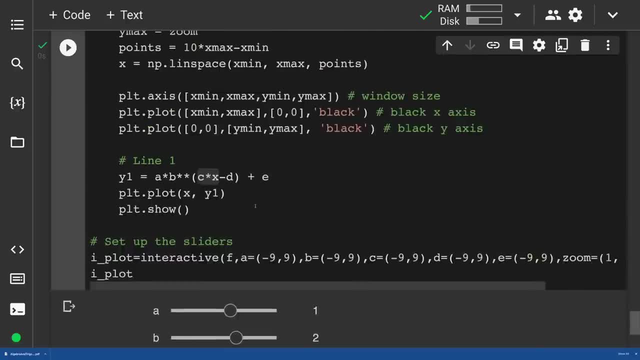 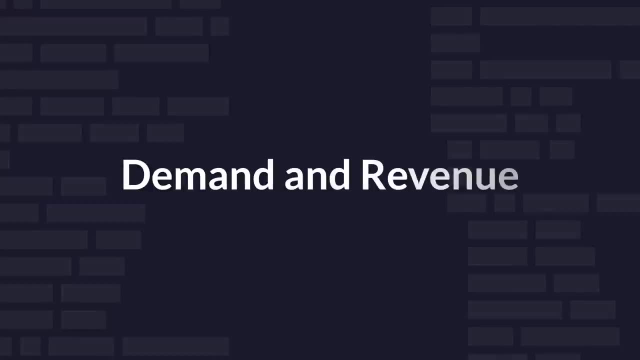 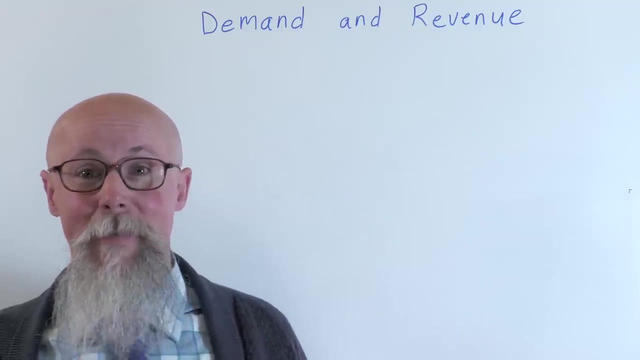 to make this show something. so we see, you know again general parent graph of our exponential function and all the things we can do to shift it. so, applying some of the formulas we've been talking about in algebra, we can use these for business applications. so, applying some of the formulas we've been talking about in algebra, we can use these for business applications. 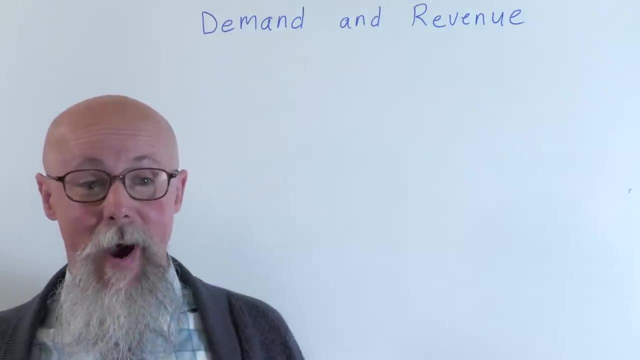 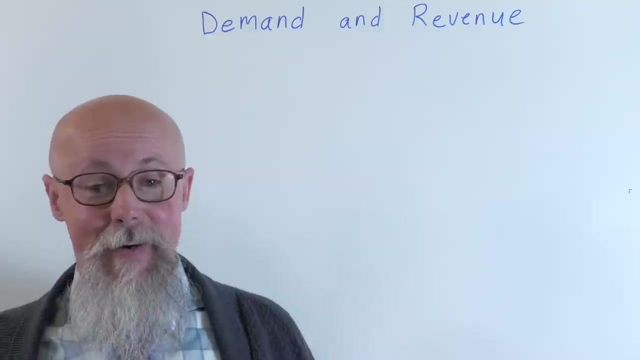 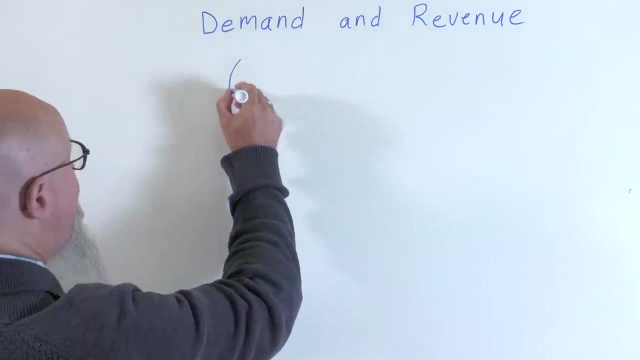 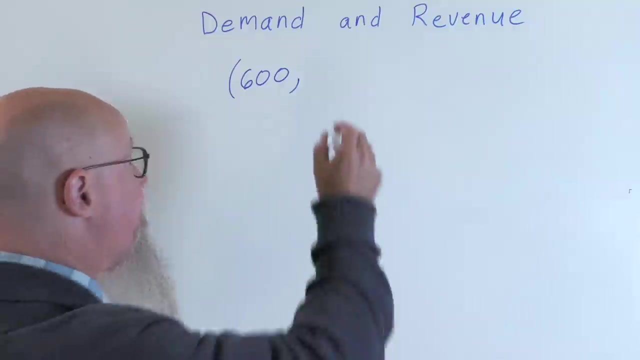 like demand and revenue. so demand would be: how many would i be able to sell? so imagine if we're selling laptop computers and i find out that you know um, an average price of like six hundred dollars will get me. you know i might sell like 84 million computers will get me. you know i might sell like 84 million computers. 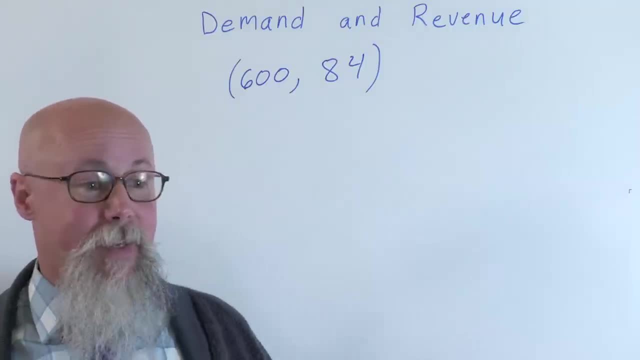 so we do some research and we find that you know, this might be the case. and then maybe i find some. some particular companies might say: oh well, you know what our average price is going to be triple. it's going to be somewhere right in the neighborhood of eighteen hundred hundred dollars, but then maybe they'll only sell like eight million. 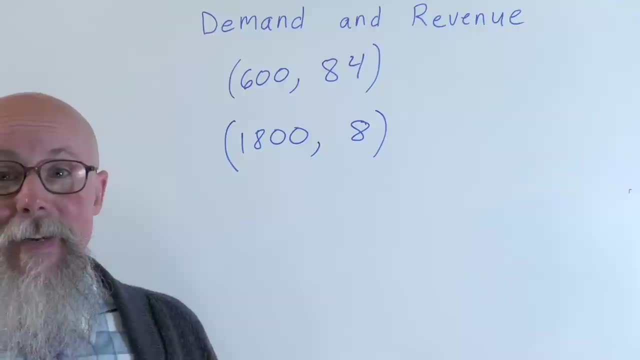 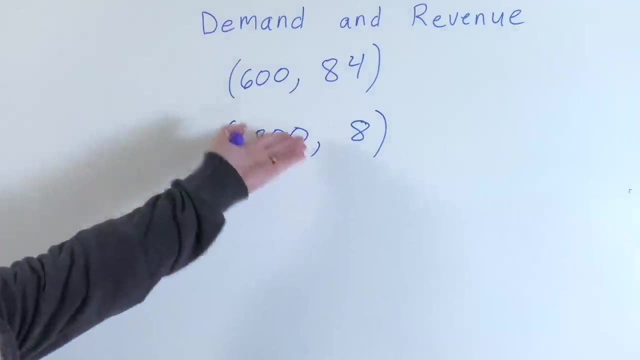 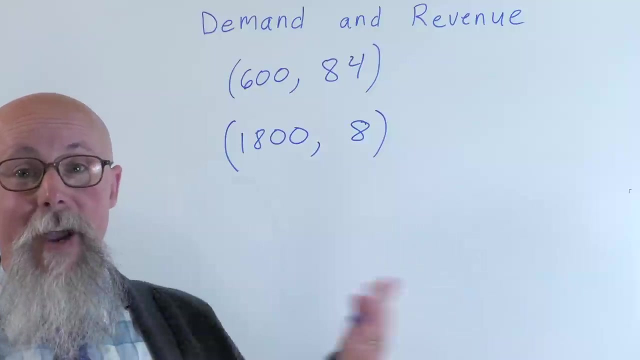 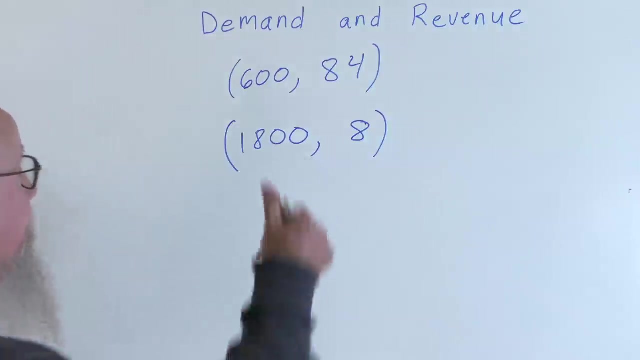 and then we look at this and we say okay, well, what should my price point be? and we can find this. we can use these two, as you know: an x value for you know uh price and y value for how many sold. and we can do the slope formula and we can get an equation here to estimate this as being linear and i can take a look at what the demand might be. so i could do the slope. you know, eighty four minus eight. 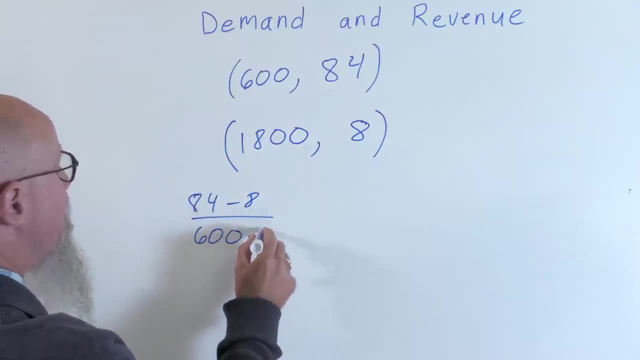 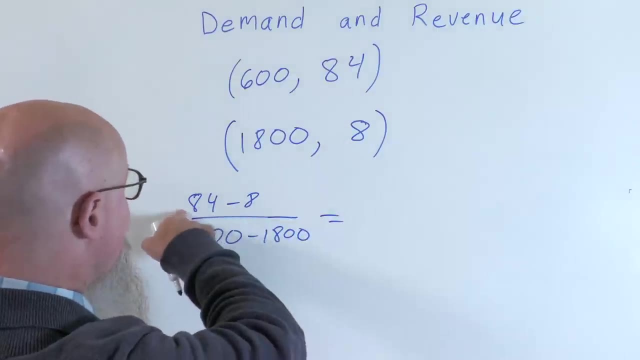 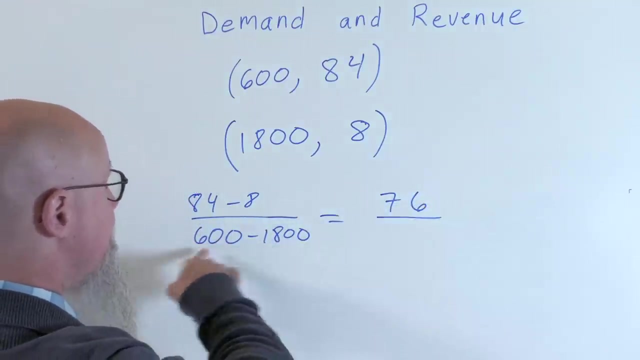 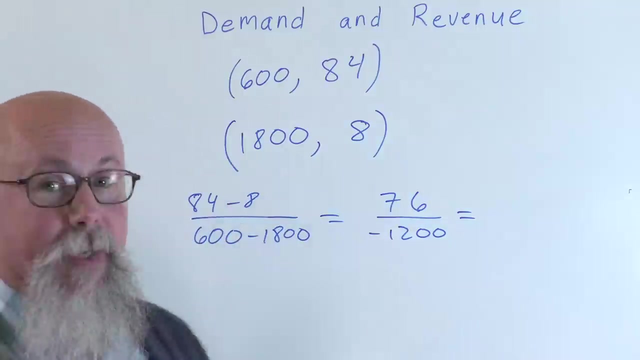 over uh six hundred minus eighteen hundred. so the denominator happens to be negative, negative twelve hundred, and i would get that into an exact decimal. that would be my slope uh, And you know it's going to be something like negative 0.06, so then I could get that into a y equals equation. you know, somewhere around there, negative, you know, 0.06x plus, and I could have the. you know what would be my y intercept. 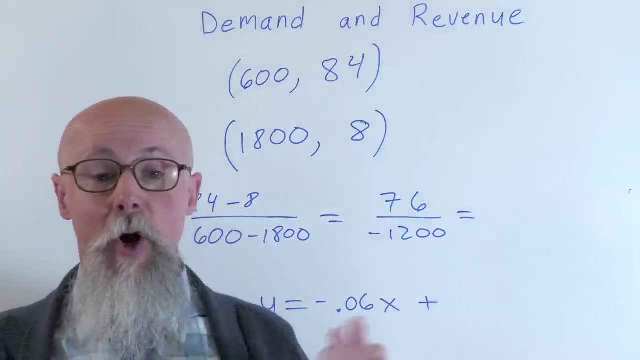 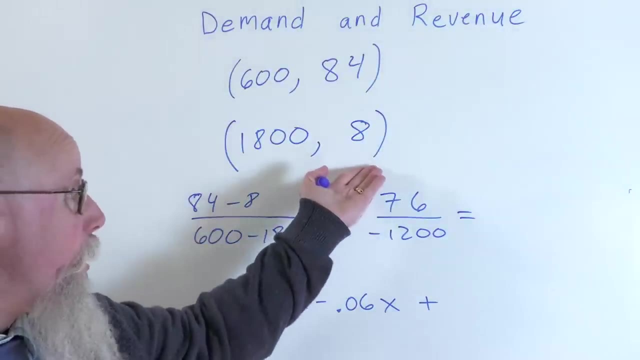 I could go through that same formula and when we get into the code I'll show you that we can just bring in these formulas that we already know, getting a couple points, getting our slope intercept form, and then I would have that value here. 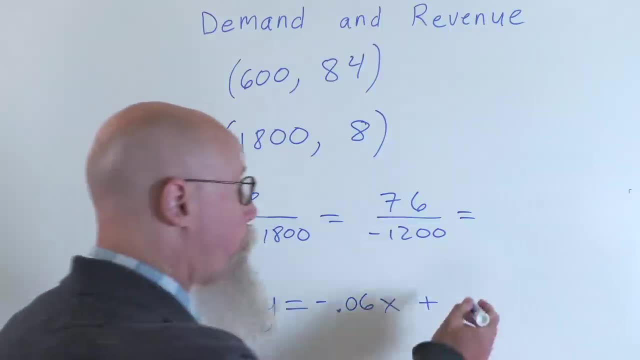 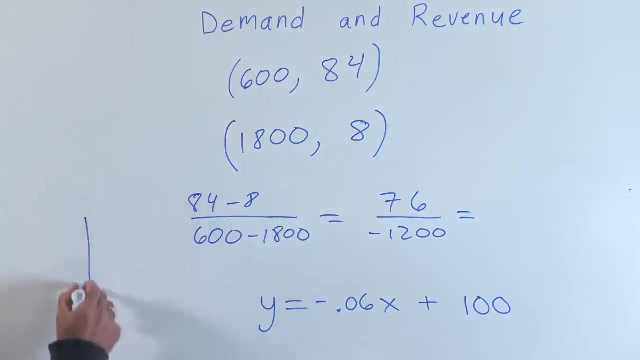 There we go and yeah, it's probably. you know I'm going to just rough estimate here, So let's just say that that would be it, And then that would be: notice, a negative slope, because as the price gets higher, you know, we would graph this as you know price and you know number sold, and we would see that as the price gets higher, then the number sold would be, you know, less and less. 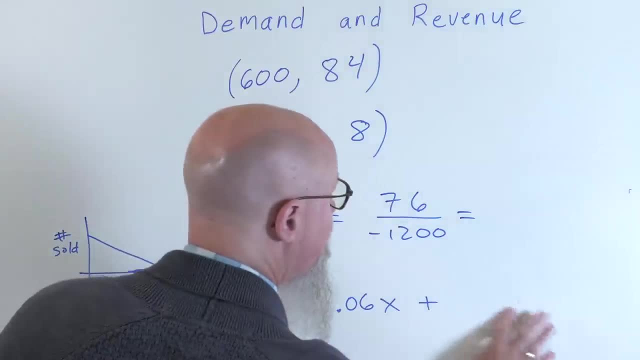 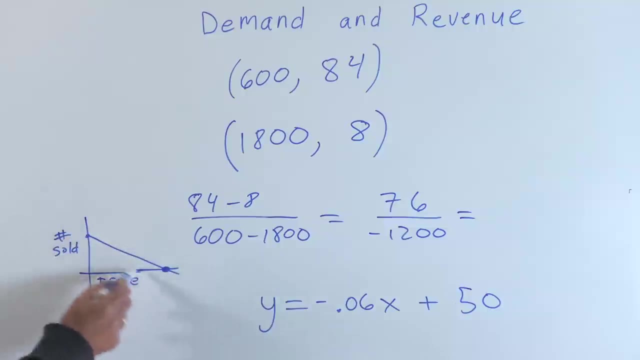 And at some point actually, the line is somewhere more like 50. And At some point, you know we the price would be so high that nobody would want it, but we would get that as the general estimate. Now let's just say that's the equation here. 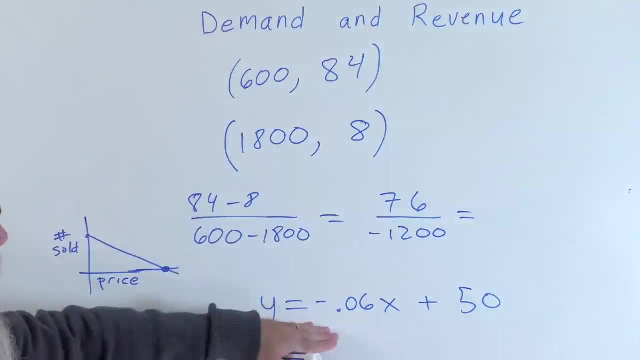 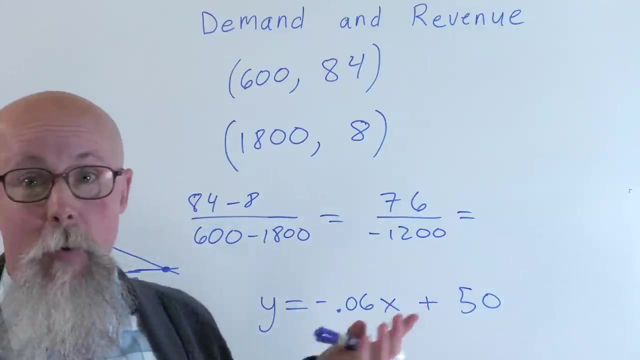 Now what? so that would be the demand equation, and a lot of times economists are looking for that. you know business owners too. What would be my ideal price point? Well then, if I use that, how? what can I do to figure out my revenue? 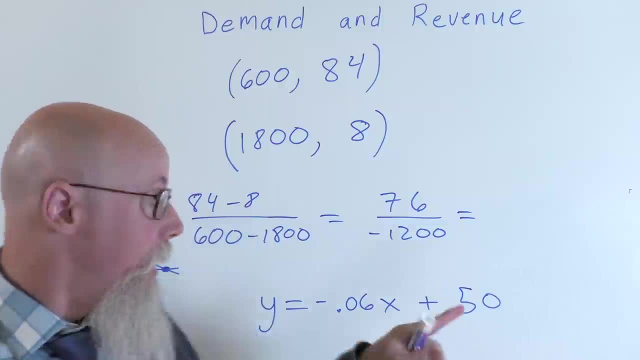 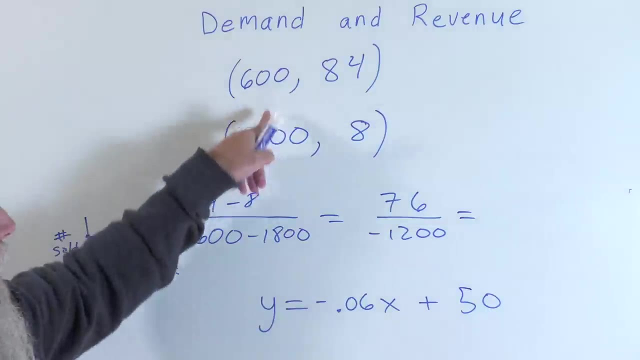 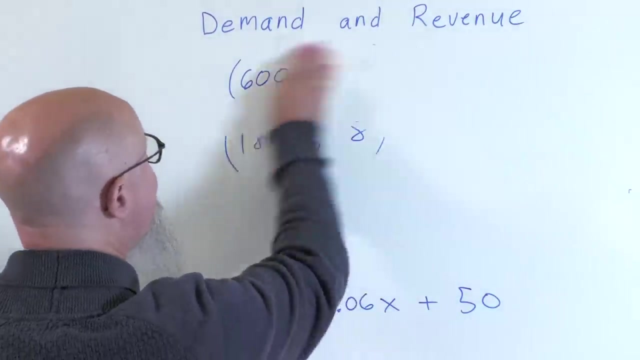 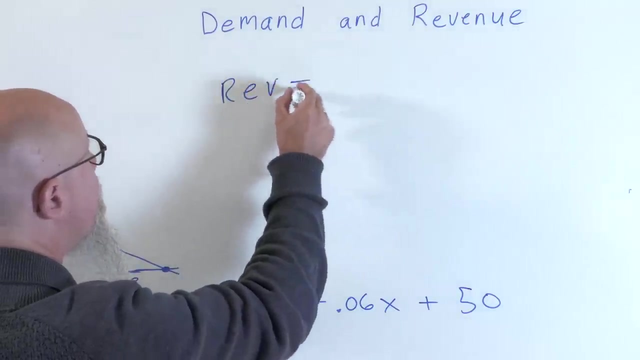 Well, my revenue, how many sold, would be the demand. but then the price, as I was saying, is defined as the X value. So at every point I would get that the X value, that the revenue is going to be the price. 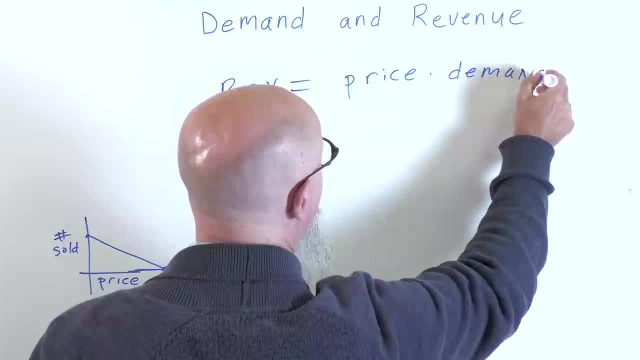 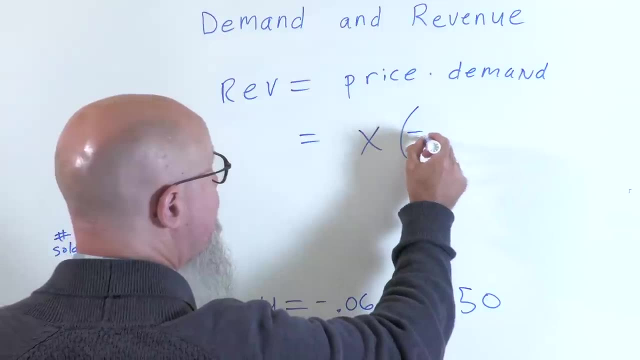 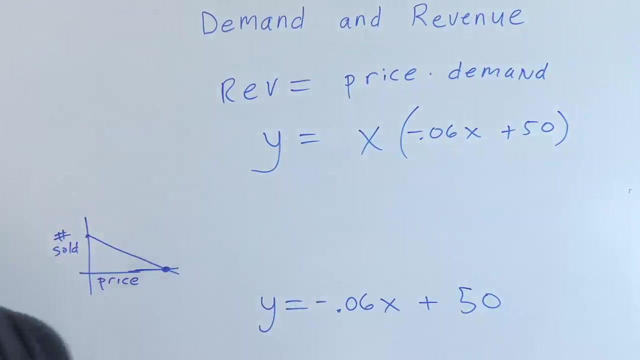 And in this case that price is always going to be X and if I figure this out, then it's X times negative 0.06X plus 50.. And you see, that would be my Y value. that I could, that I could graph. 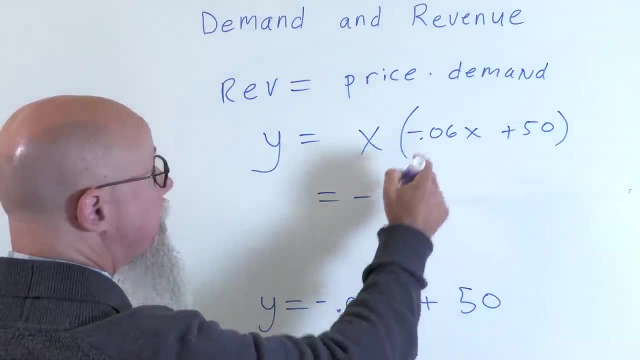 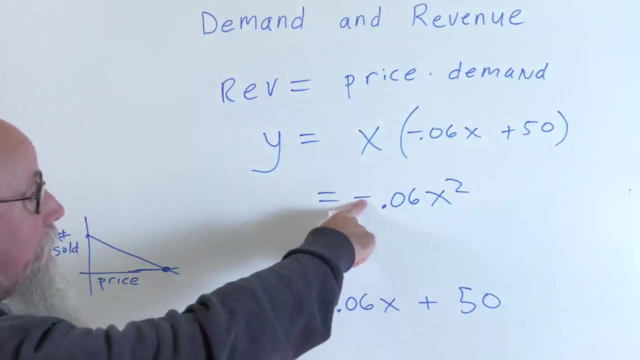 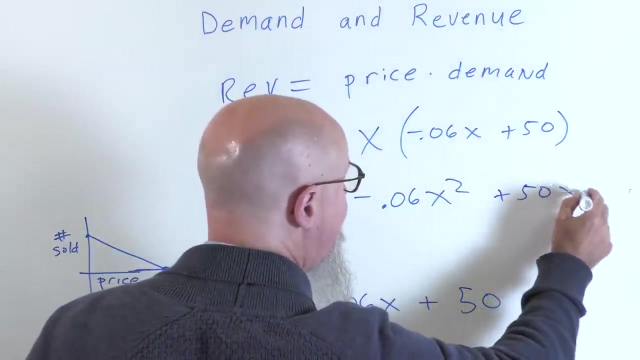 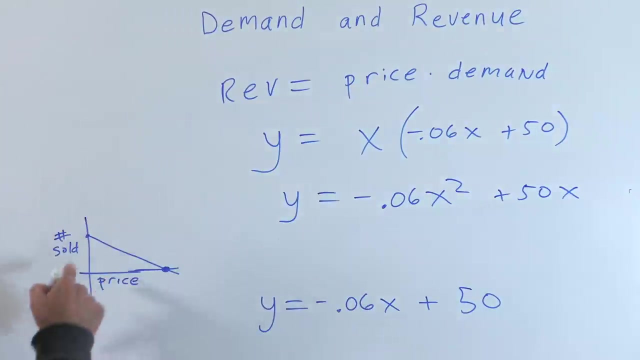 Quick distributive property. we recognize that this is A quadratic with a negative A value, so that means it's going to open down, you know plus 50X. And so when we look at this, then if I have you know the price, but then instead of the number sold I want to have revenue. 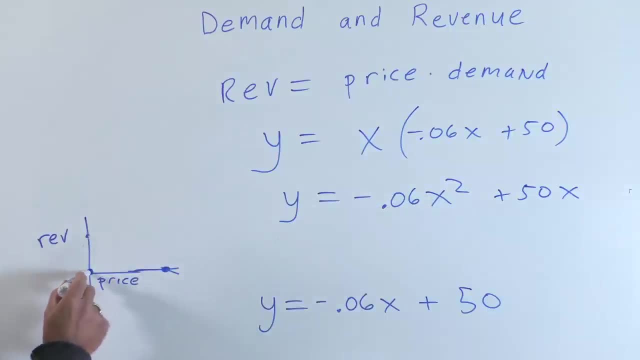 So, of course, if the price is zero, I have no revenue. and then of course, there's some other price that is so high that nobody buys it, so I have no revenue, and the shape of this graph is going to be a parabola that opens down. 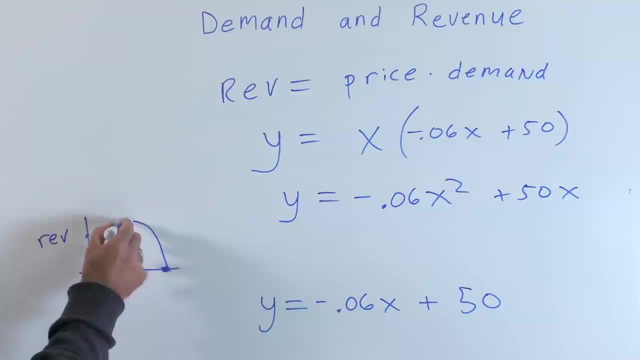 So then I see that there is some middle price that would maximize revenue, and that's kind of the thing that we want to look for. You know, using these formulas, we're using the slope formulas, we're using the formulas we've developed to generate a slope-intercept equation. then we're using this like this would always be true: revenue is price times demand. 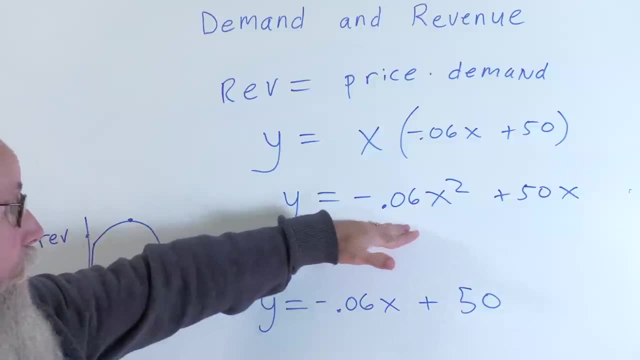 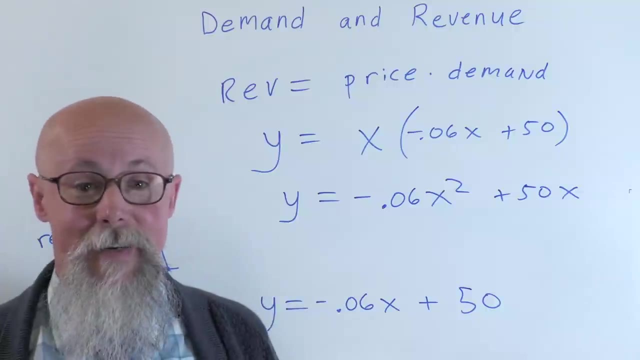 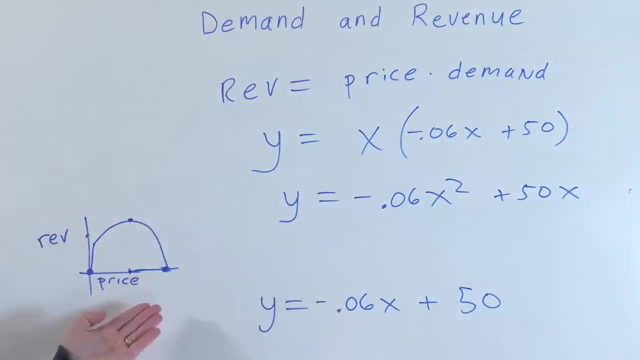 So then we can use that to develop this quadratic and we can graph these, we can find out what these, what these revenue points would be So pretty interesting. Then we could also apply this to price. So this is just revenue. and then we could do this and then subtract, subtract the total cost, we could get profit. 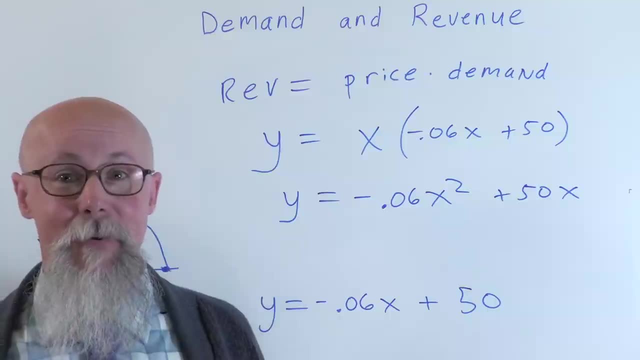 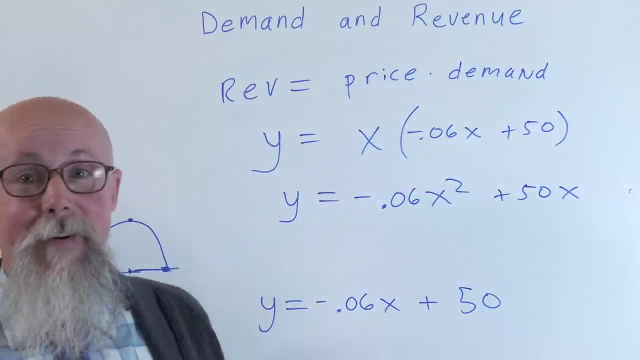 So this is really some of the applications that we want to get to that you know, using these formulas and determining based on some data. you know, what should my price point be? to maximize my revenue Or, given you know, if I already established a price point, what would you know? can I predict the revenue? 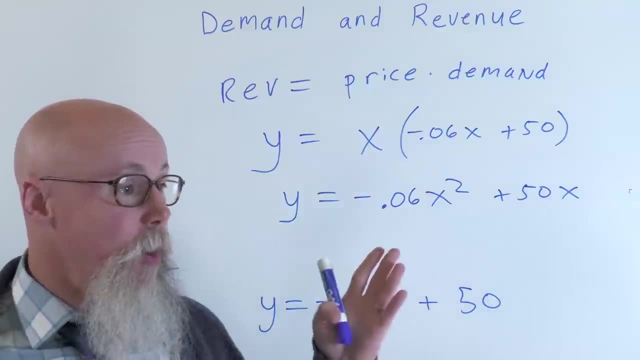 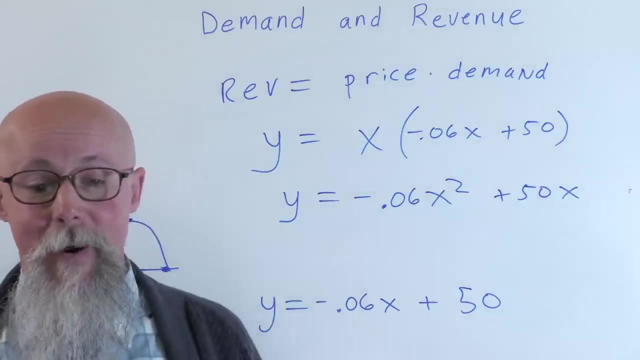 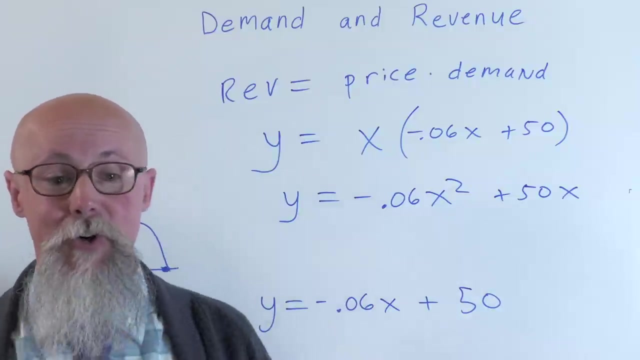 You know, these are things people put in their business plans. So we see these examples, or this one example, and I, when we look at the code, I have two other examples so that we can see how this would come together. that you know, you can use your math skills, you can use your Python skills to make some business predictions. 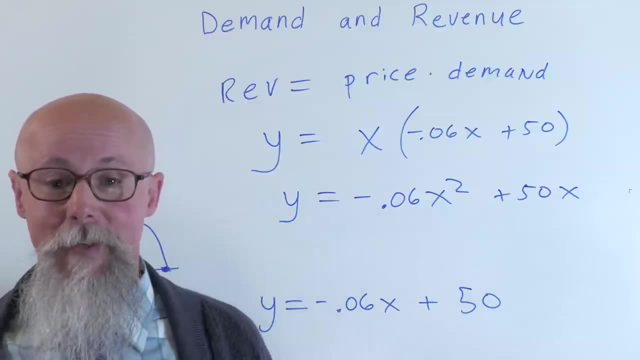 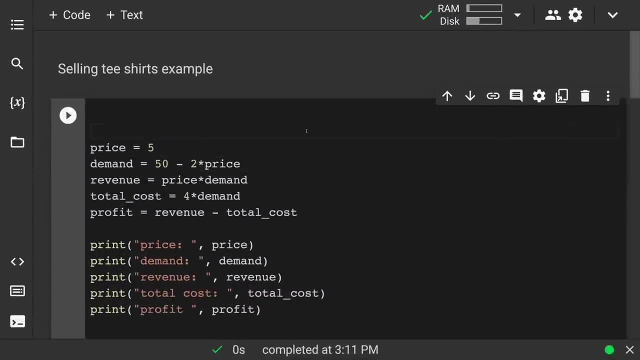 And these are some of the good applications of all this math and writing code. So let's take a look at the code. All right, so I wanted to give you another example or two to show how you can write code to work with these formulas. 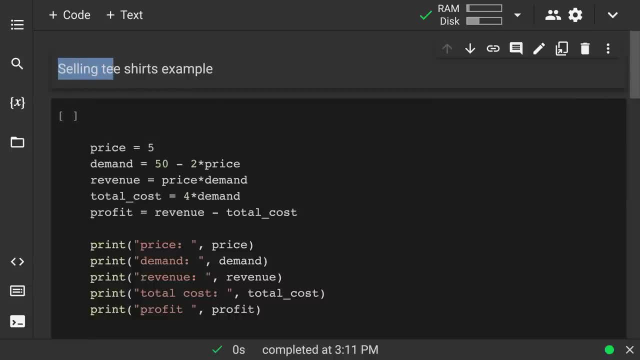 And for this example, I'm just saying we're selling t-shirts And I've made up these numbers. hopefully they seem kind of realistic, But you could define the price here, and so these are all variables here. So if we define the price and in this case we're going to say we're selling t-shirts for $5. 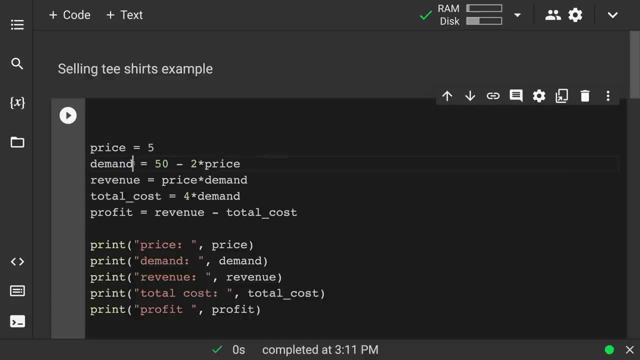 And then we have the demand as our next variable And we're saying that if you were giving away t-shirts, maybe you could give away $50.. You know, this is business, you're not really going to give them away. But then your demand decreases as the price increases. 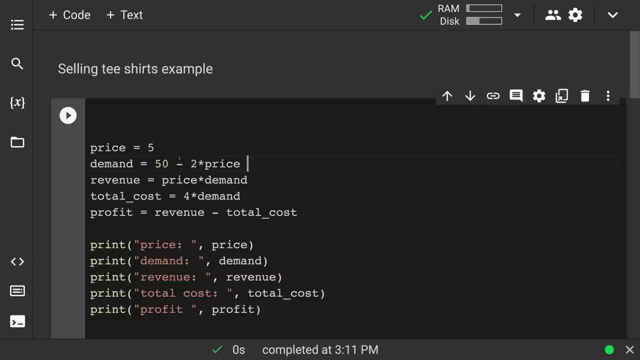 So every time the price increases. Now, in this case again, if the price, if it was free, you'd give away $50.. Right, here the price is $5. And then so two times the price is $10, so then the demand would be $40. 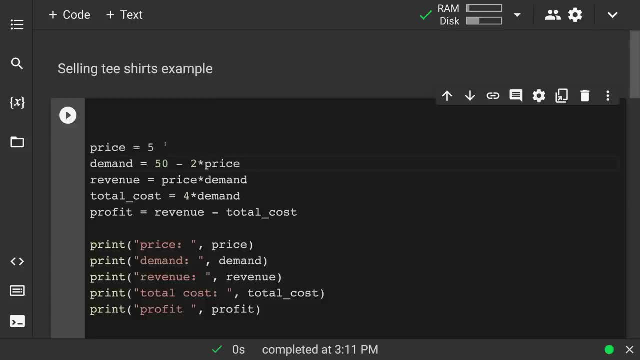 But you see how it just cascades. we just define the price and then we use that to talk about demand, And then revenue is going to be price times. demand- Now that is actually a standard formula: The price you're selling it for times how many you sold. 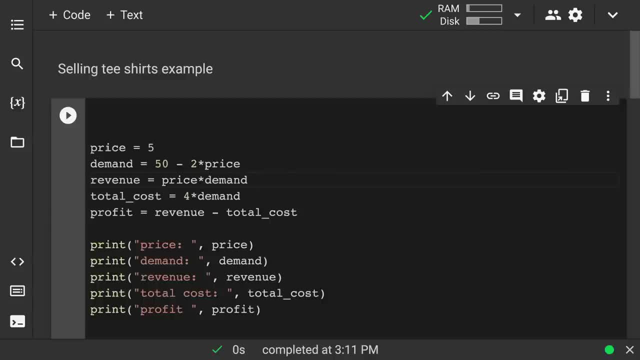 So you see, we can do this. we've, you know, once we've defined these. Then we have these other formulas that that can depend on them, And then the total cost. so this is another one that you would have to know. 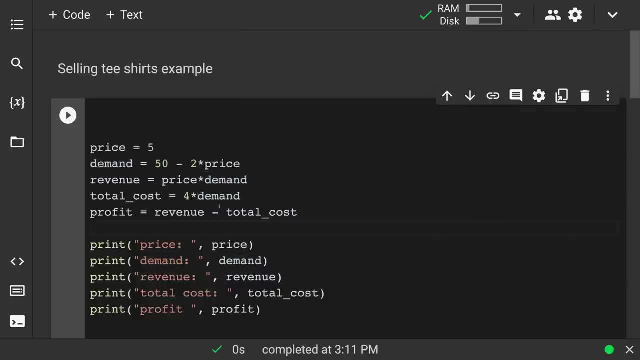 And I just made this up. I said four times the demand. So if we have four, you know, the idea is that let's say it cost $4 to make each t-shirt. All right, and I'm sure sometimes t-shirts cost less, but I just said $4.. 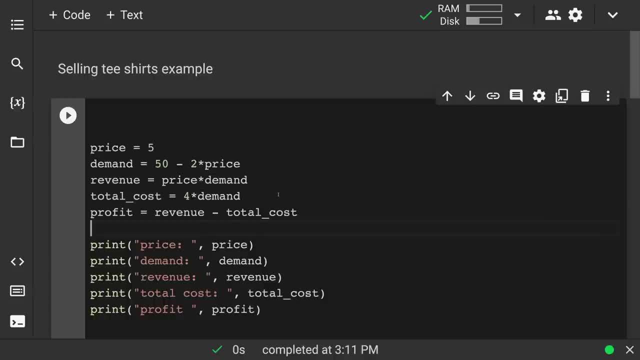 So that's where the total cost would be $4.. $4.. That's times, you know however many we sold- And then that's the total cost. So then we have: profit is revenue minus total cost. Makes sense. 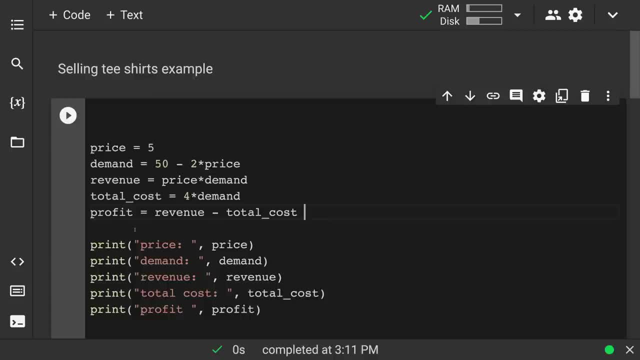 What's the rev? how much money do we bring in minus the cost, And how? you see how we have all these. we can just define these formulas. Now, this is a standard formula for for profit, Revenue minus cost, And this is a standard formula for revenue. 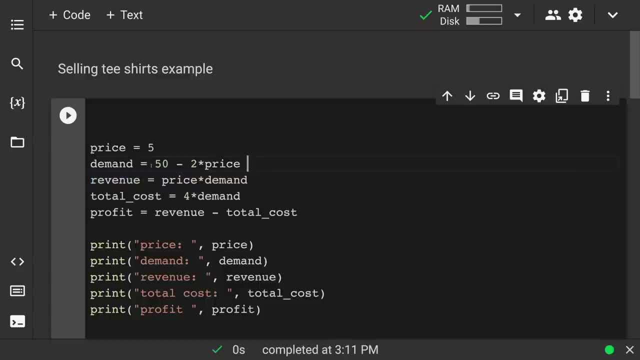 So if we can add it to some, I've got a price and these two here right here, all of these up to $6 each, And then felt price, times, demand And some of these. then we could develop these equations if we knew, if we had some other. 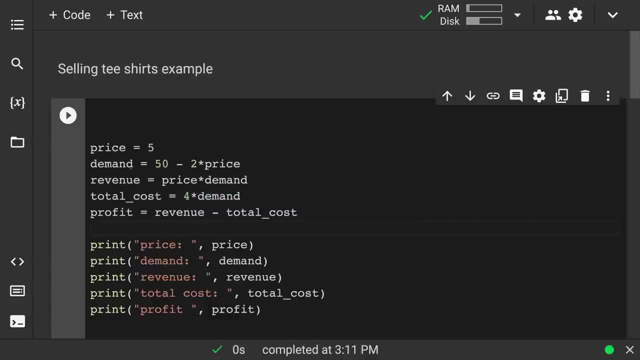 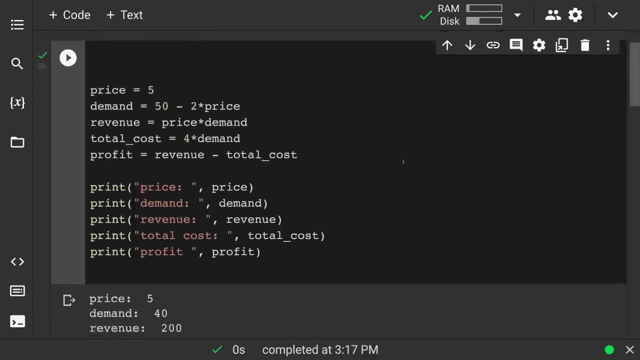 data. So if you're making things to sell, you would definitely have this information. How much does it cost to make? But there you go, All these. then if you define the price and some demand equation, we can calculate all. 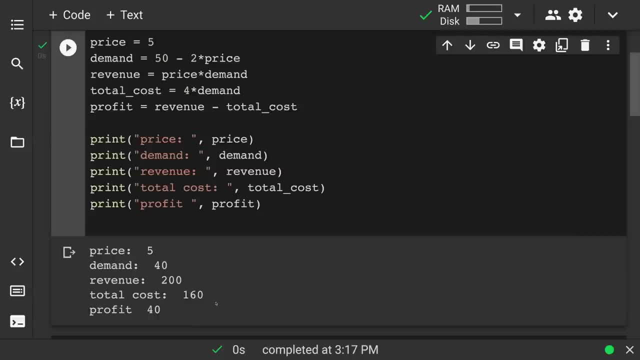 these, because 5 times 40 and then the total cost will be 160, you make a profit of $40 and then having these, this is where people can do some research and they can test things out. oh well, let's say supposing. 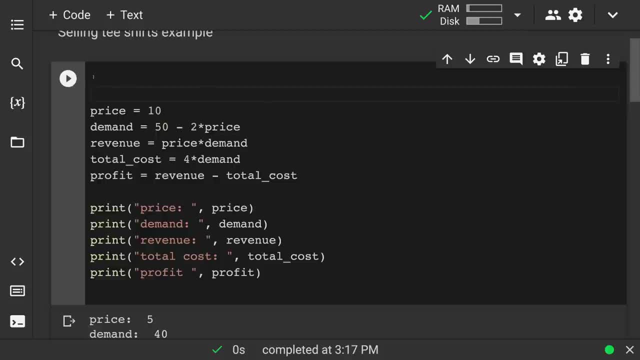 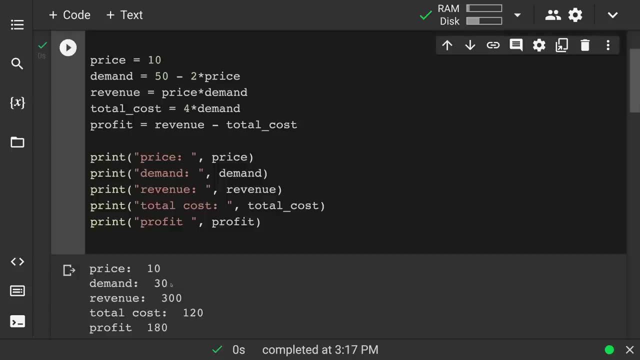 I decide to make the price $10 instead. and we take a look at this: the price increases, the demand decreases, as we expected, but the revenue increases and so, given that cost, we still have a profit of more than double. so the price of each doubled. I went from $5 to $10. 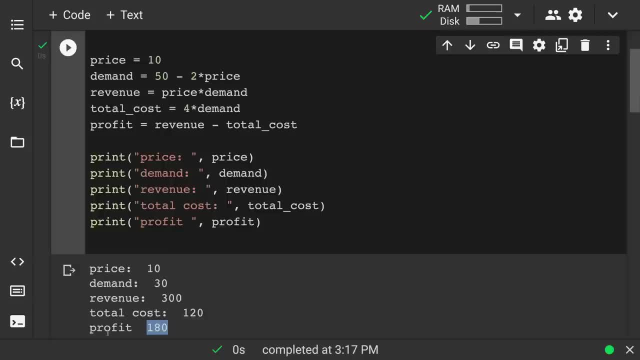 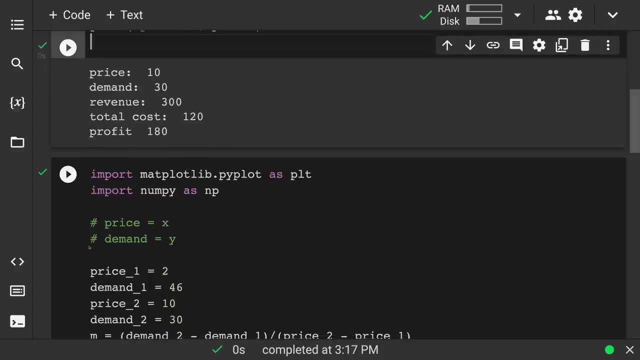 but the profit more than doubled, it more than quadrupled. so just interesting things that we can see here. and how does this happen? well, it might be helpful to see this on a graph too. so we're going to graph these things. import matplotlib and I'm going to import numpy. 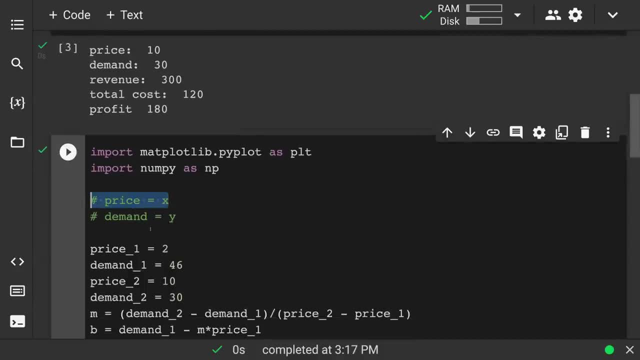 I'm just going to remind you here that the price is x and the demand is y, and then we're going to change it that the demand later is going to be the revenue. now, this is where, if you had data, this is where you would have. 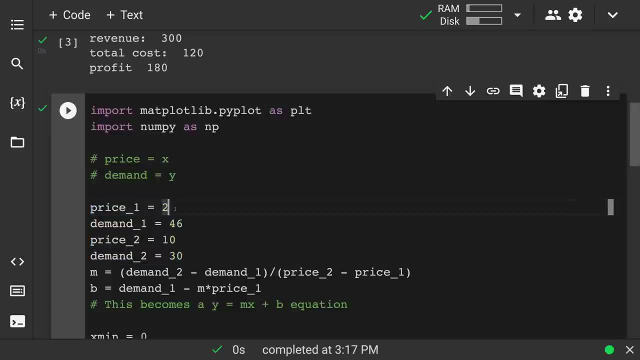 if I have, at what? at a certain price, what would the demand be? you see, and I had in mind here, you know that this was, you know, I don't know something else. here you're buying $2.46, so it would. it might not be t-shirts. 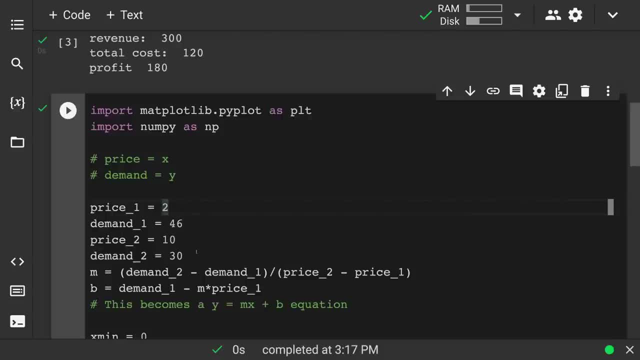 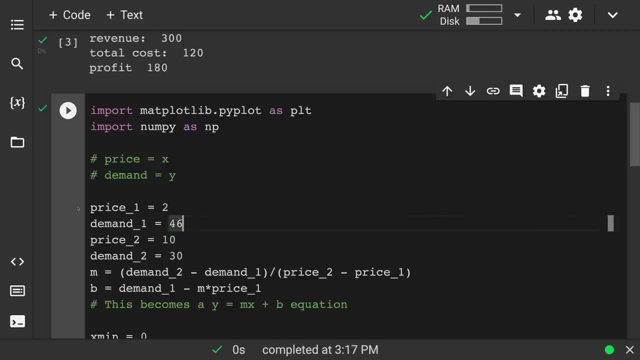 demand. so it's something else that you, you might have. but there we go. so we can define these: price one and demand one. so if it was two dollars, then the demand is 46. if it's 10, then the demand drops down to 30. as an example, if just having some of this data from some other research and we can 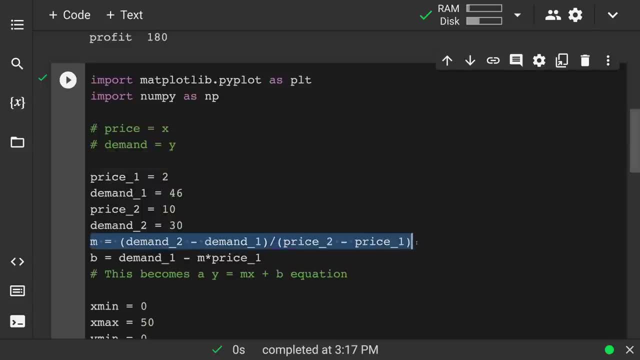 remember these formulas. we did back with linear equations because this is essentially two points: price and demand, or x and y. so i'm going to calculate the slope based on those two points, calculate the y intercept and then this becomes a: y equals mx plus b equation. so pretty cool. 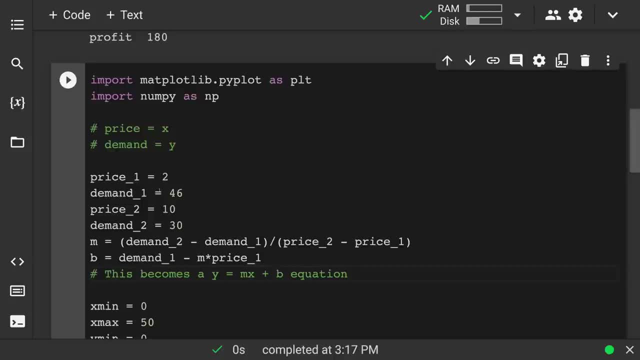 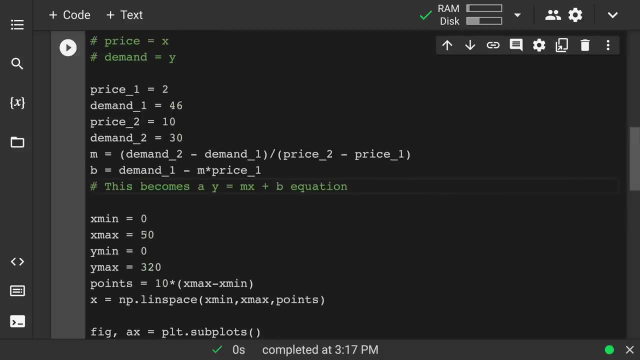 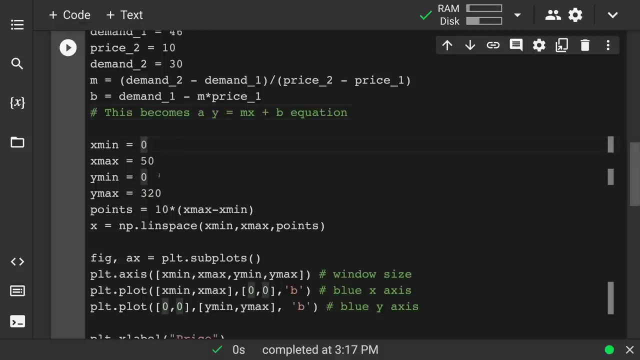 again, if i have, you know, some examples of some data that we have that we can, we can test. so, given that equation- that's going to be my demand equation and i'm going to go through there- we go x min, x max. now notice this: x minimum and y minimum. i'm going to make zero because negative. 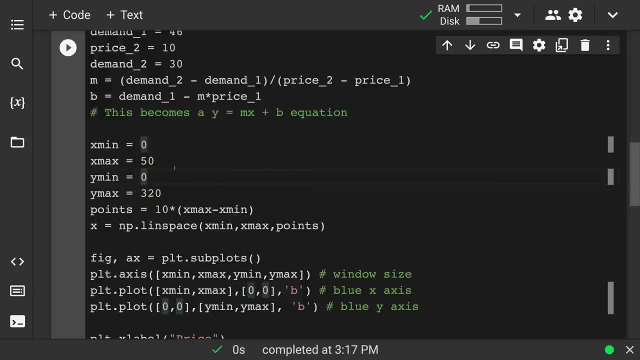 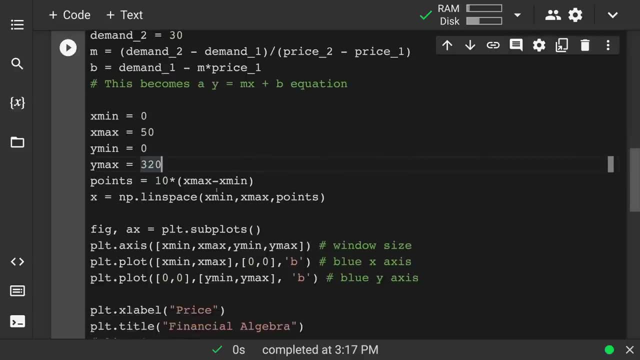 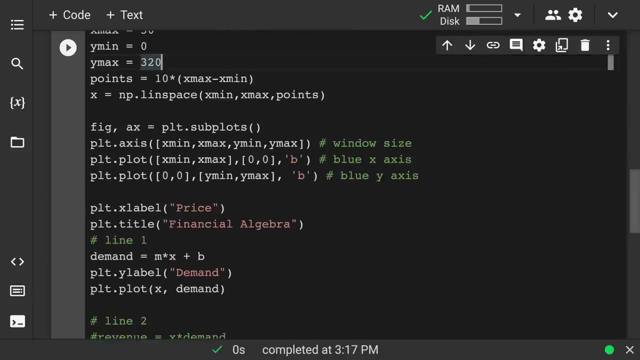 numbers for this aren't going to really have any practical meaning. i'll make the x maximum 50 and y maximum 320.. there we go, the number of points. that's all fine. so after i define everything here, i'm gonna do a couple other things. i'm going to do the x label is going to be price, and then i'm going to give. 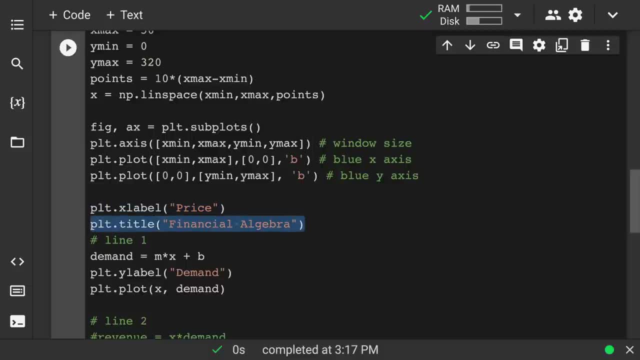 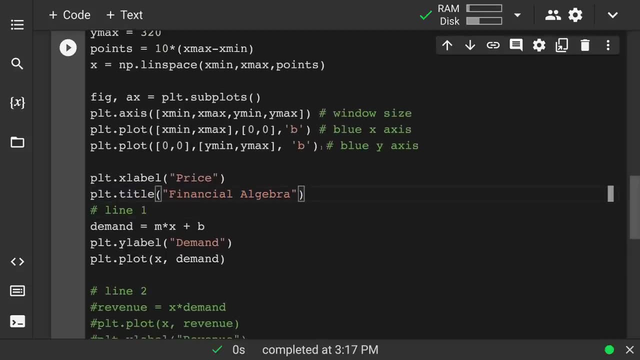 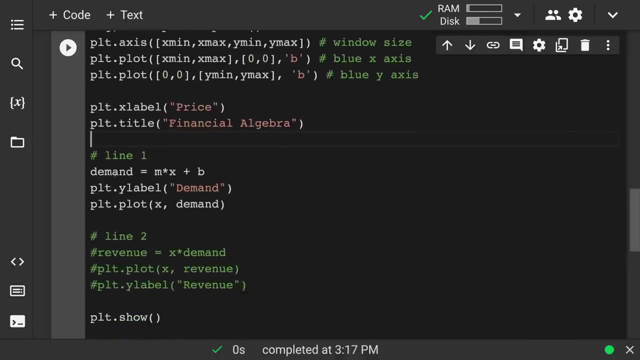 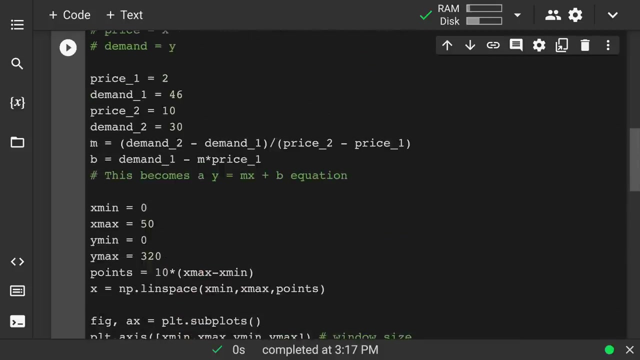 my graph a title. so notice both these pltx label, plttitle. there we go, and then for this one line one i'm going to have. so for line one, here's my demand. equation: y equals m, the demand equals m, x plus b, and so we figured out m and b up here. 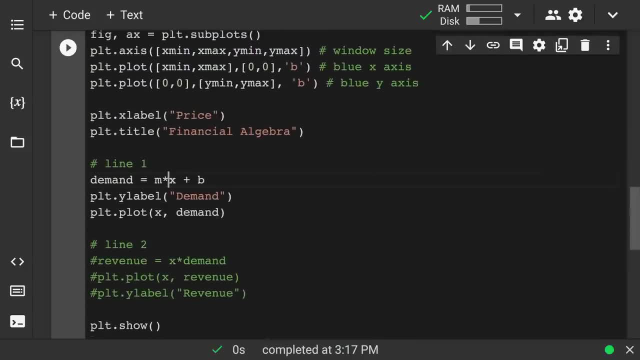 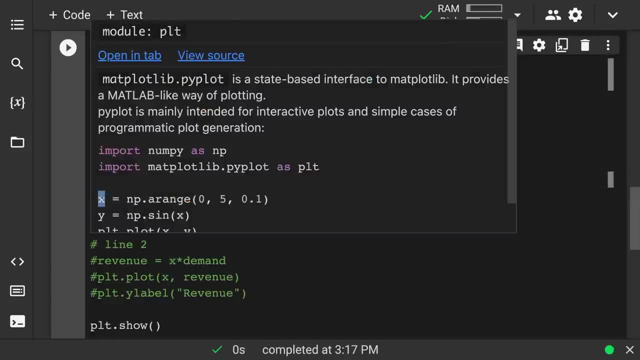 and so i can use those, but i'm going to use x, because that's the array of x values that i've defined. so we have our demand equation and then i'm going to plot y label, demand. so we see the x label is still going to be priced, but for this one y label is going to be demand and then y labDay mean. so 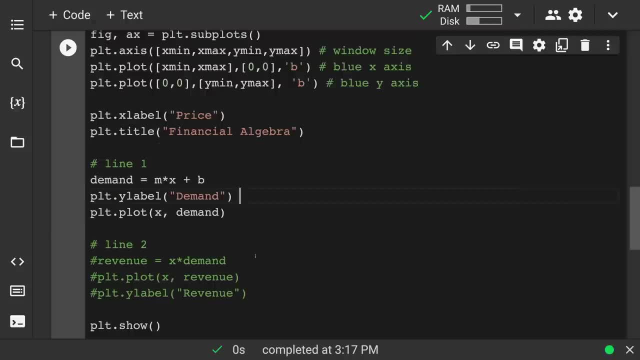 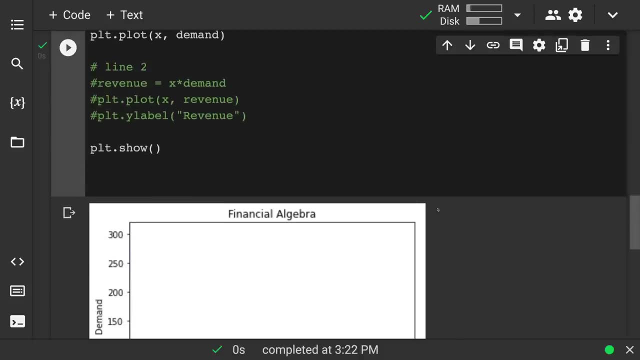 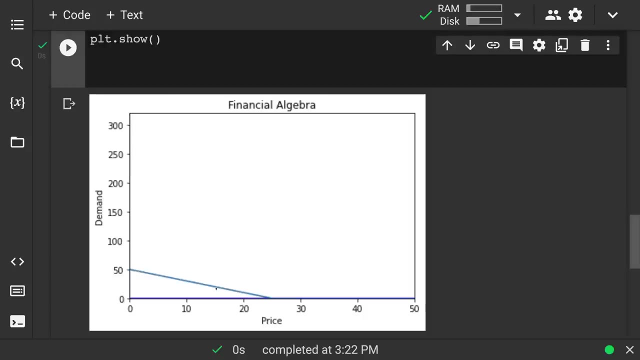 was going to be demand. and then we're going to plot x and then the demand. i commented this out, we'll get to that in a second. so here we go. so i have my graph. and then we see: yes, if i was giving them away for free, i could give away 50. the demand decreases as the price increases, so at some point, 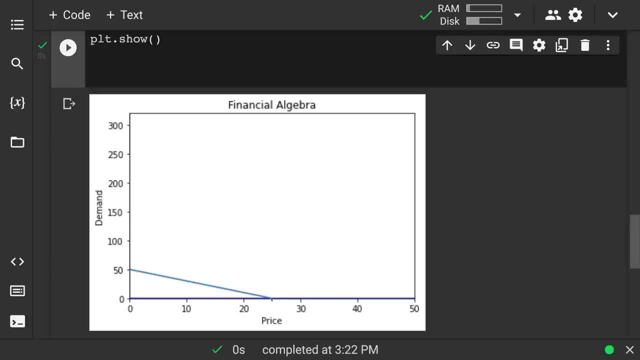 maybe like 25. um, you know, whatever i'm selling here that started out as two dollars. um, you know, maybe it's cds or something. you know, some people still want those. um, if i have 25, you know, nope, too expensive, nobody wants it. and then somewhere in there we have the ideal. um, now, it's not always. 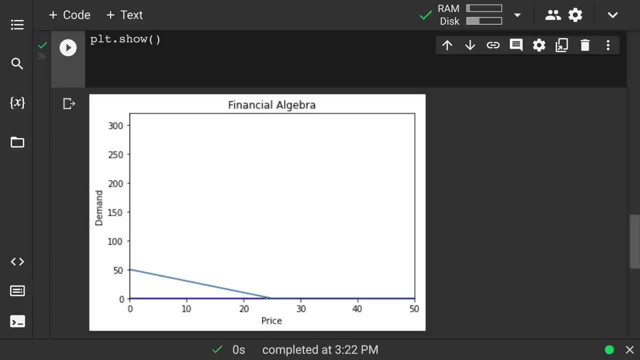 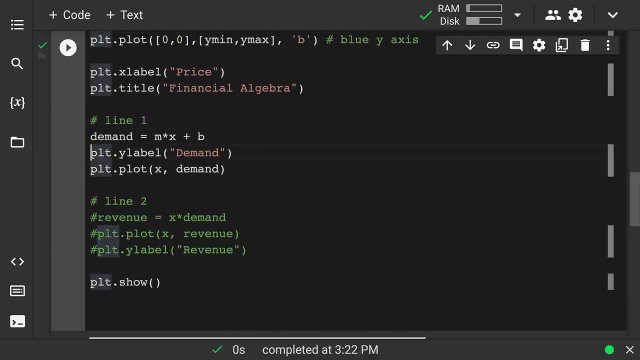 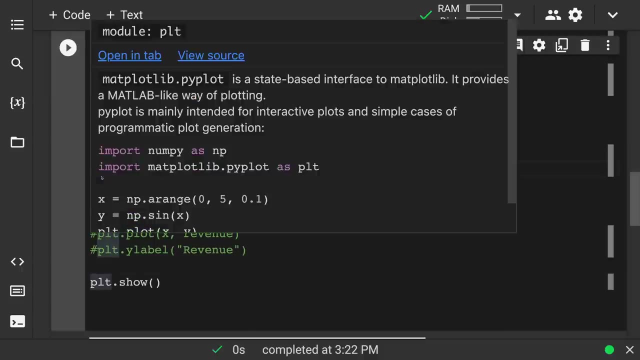 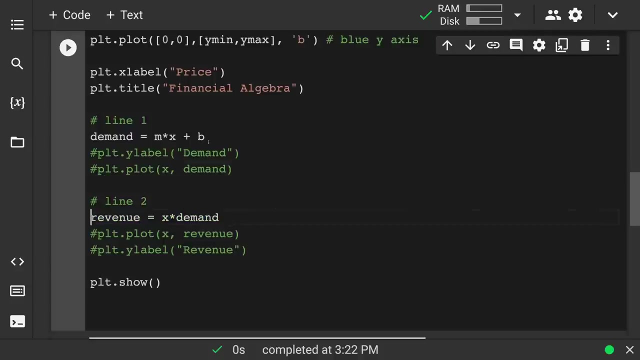 perfectly linear in real life, but this is a good estimate. so, given these- supposing i keep that same demand equation and, as we were saying before, i can build upon that and i can have revenue equals x time demand, because as long as i keep that equation, it will still use that and then. so now i'm going to plot my x value and then revenue. 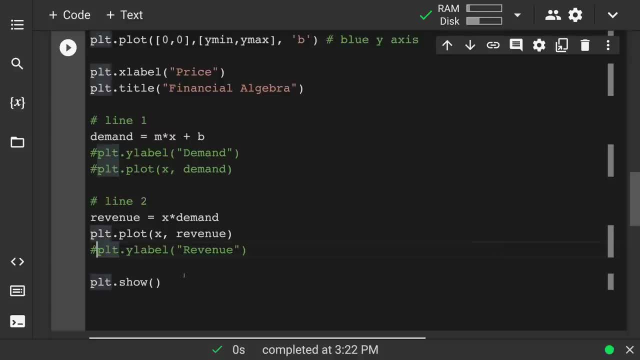 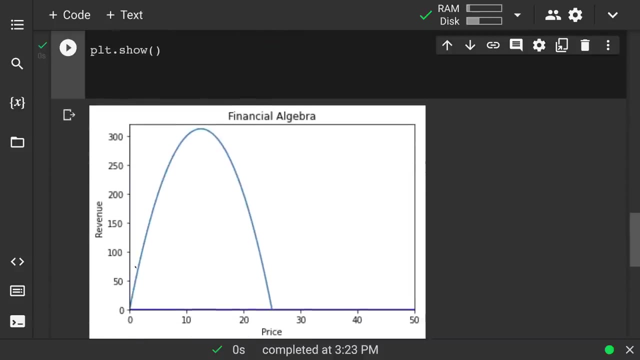 as Y value and I'm going to change my Y label to revenue. so we see that we have a way to do this. and when I graph this, we see that, yes, of course I'm going to make no revenue if the price is zero. and then we said that about 25, I'm going to 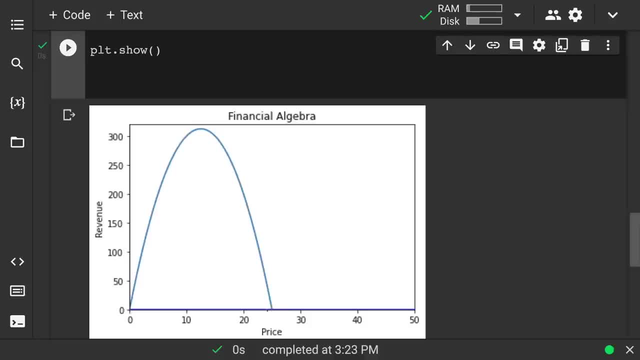 sell none, so that'll make no revenue. but this is how the revenue goes and it's really interesting that I can have some. you know low prices and I think that that's you know the best. I might sell the most, but the revenue actually there's some middle number here that gives me my maximum revenue and you see, 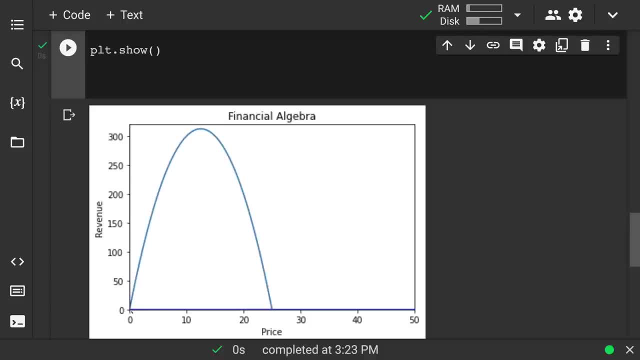 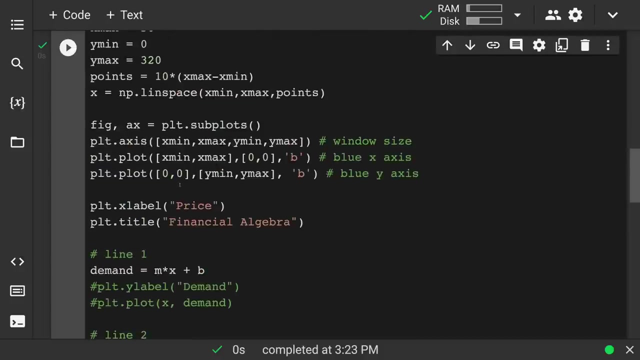 it looks like now: if, if I make new revenue at zero and at 25, these parabolas are symmetrical, So it's exactly 1250 would be the maximum revenue. or, if people like round numbers, you know 12 or 13.. So there we go. we can see how we can use all of this and we can. 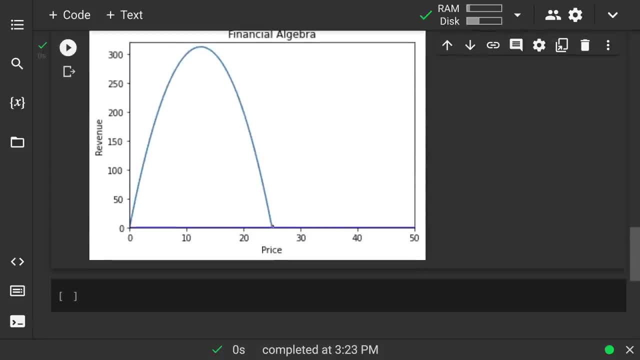 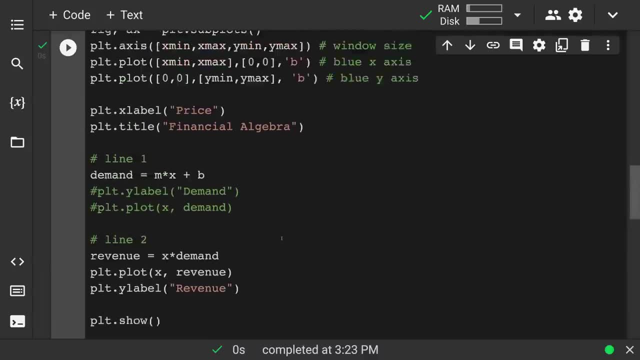 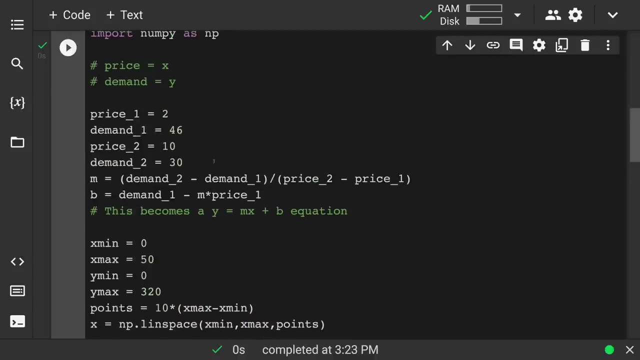 see that the you know the reason why revenue would be zero here. this is where the demand would be zero. So this is probably the more. the line two is probably the more valuable one, But having give it, getting some research of given prices, demand, price demand that. 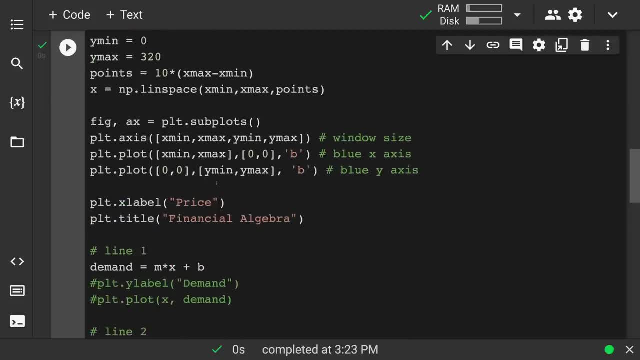 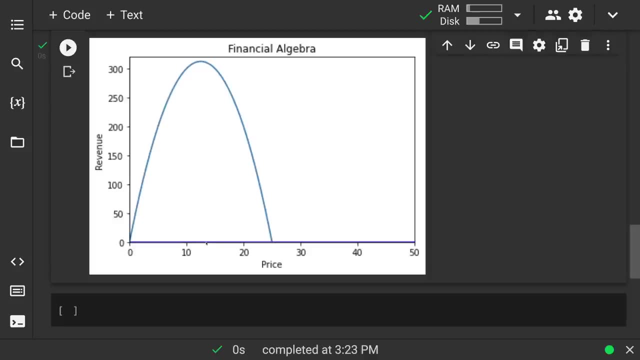 if I have a couple values here, then I could plot this out and I can plan, Oh, from other prices and demand research that I've heard. what should I make my price? You know, and this, this is some of the research that people can do, You know. 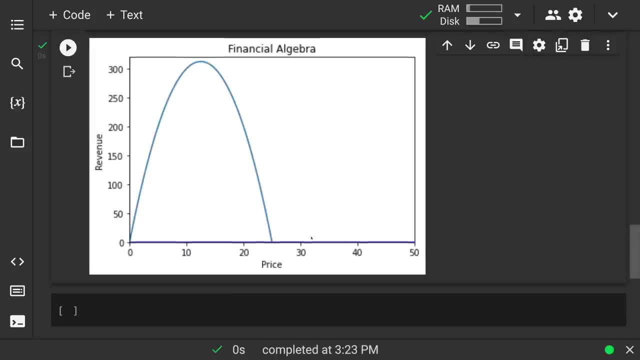 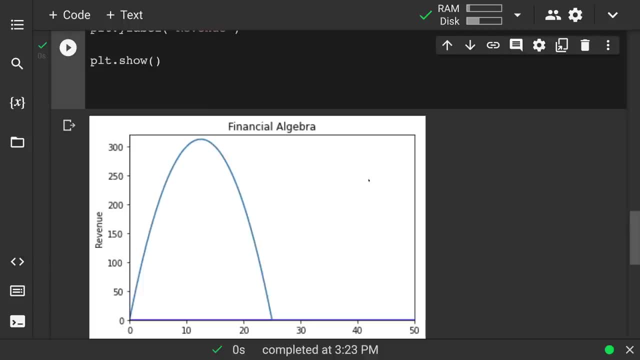 you have some new product, how can you determine what the price should be? All right, Next slide, There you go. Have also. then, if you're making a business plan, you could always then download or export these images. you know, you've, you've written the code. 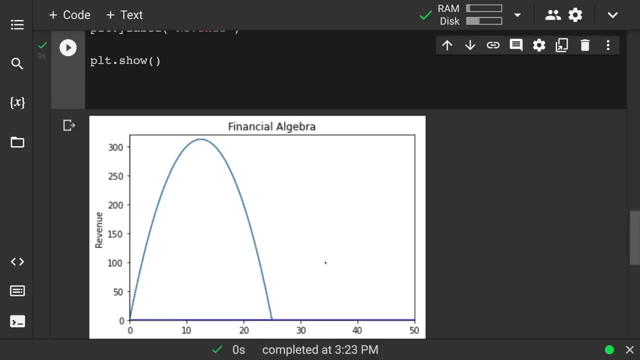 see the graph, export the graph as an image to include in your business plan. So there we go. You know a couple different examples of how we can make use of these. you know formulas, the graphs, and generate some graph or some image and some data that we can really use. 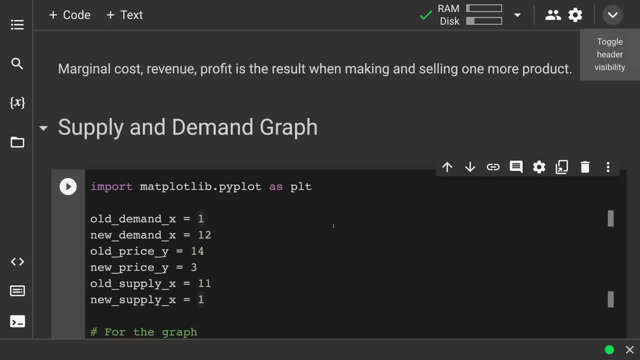 Okay, so let's apply some of these graphs to some other economic theories and see how you can use Python or math to plan predict. look at trends in economics. We looked at cost revenue, profit and if we take on that marginal cost revenue or profit if it's marginal. 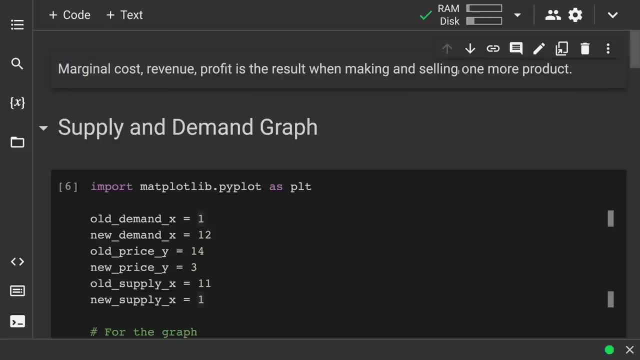 then that's the result when making and selling one more product. And for some of our examples we were doing some linear equations and for that the marginal. if cost is linear, the marginal cost is going to be the same wherever you are. But sometimes we have 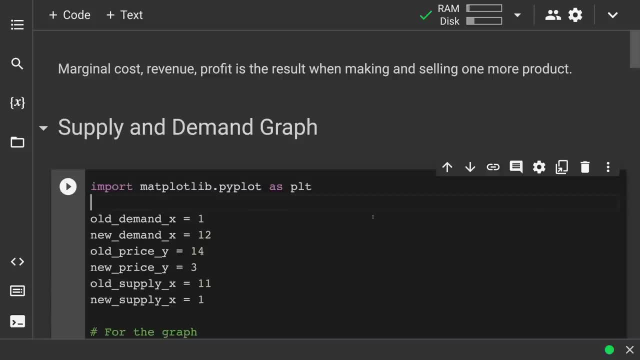 costs, or we saw that definitely. we have profits or revenue that are not linear And therefore we have some times when- oh, this is, it makes more sense from a cost, revenue, profit perspective to make one more, And sometimes, you know, it doesn't. Sometimes 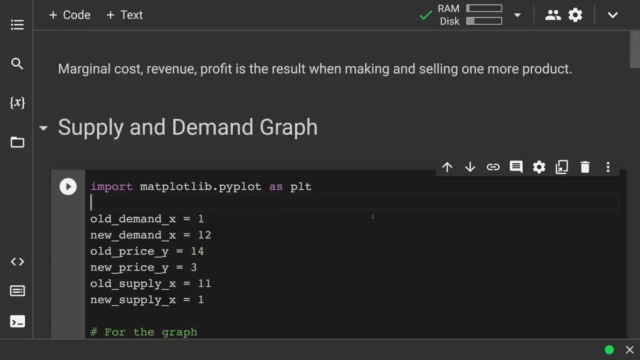 you know, oh, that one more is only going to get me a tiny bit of profit, Not worth it. And cost. sometimes it goes the other way. you know, setting up everything, making one product might be a really high cost, but now it's all set up, So making 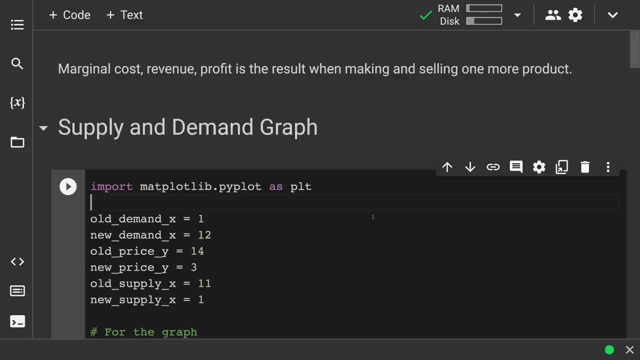 two, three, four, a hundred thousand, you know might make that worth it. You know things like newspapers and book printing and you know there's a big setup for the printer And so the marginal cost to make one wouldn't be worth it. Now there's definitely, you know. 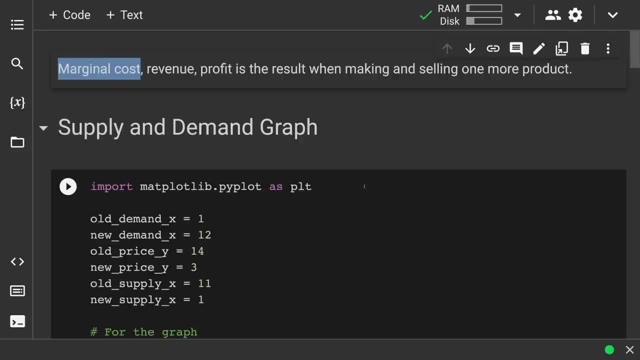 other methods, printers. but for a lot of the big printers, like a newspaper, marginal cost it'd be a whole lot for one newspaper. but no, they're going to print thousands and thousands. So the marginal cost after they've printed, you know, a hundred thousand. 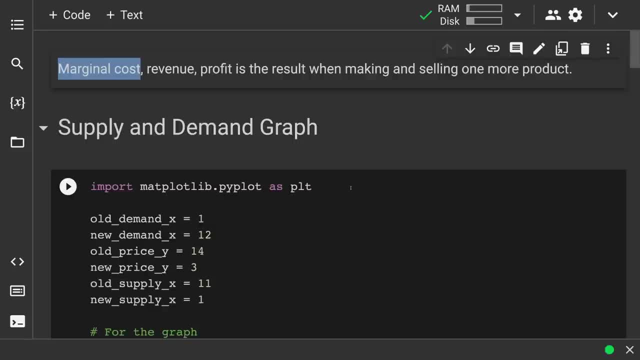 newspapers. printing one more is almost nothing as far as cost. So these are the things. you know what. what's it cost to make one more, And you know we might notice that for revenue and profit the same thing, And so if we have revenue, you know. 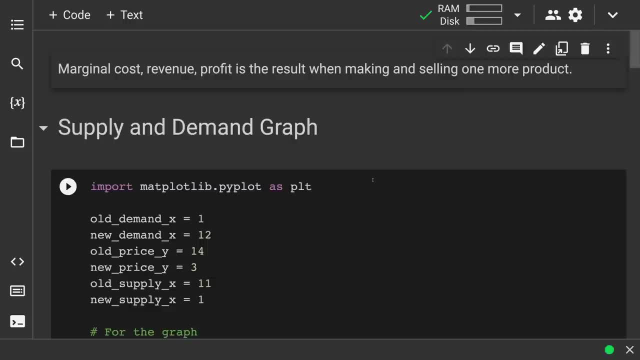 and this kind of a lot of times comes up, you know, toward the end of the day people say, oh, what you know. what would it take to make one more sale? You know, maybe it's a store. Should I stay open for? 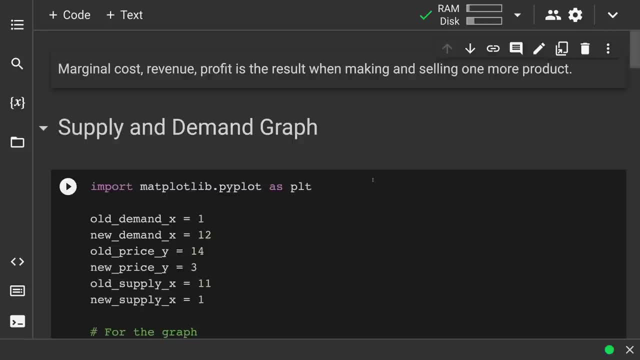 a lot longer and everybody's tired to make one more sale That might be, you know, a lot more cost to in a lot of ways for a little bit of revenue, not worth it. And so they say, okay, these are the hours when we. 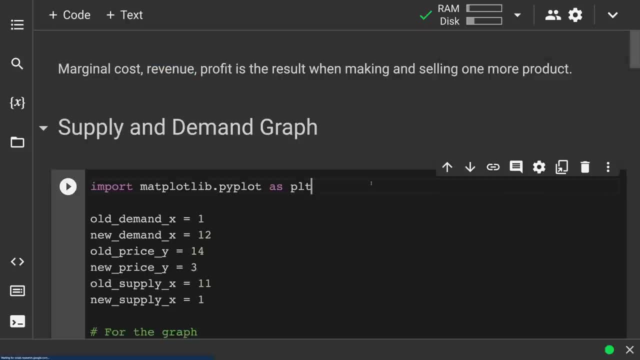 close. So these are some uh, deeper analyses. as we get into things beyond linear equations- Um, we can do even more of them. That makes that even more interesting, but just to mention that, you know, as we talk about this, the marginal is that at any given point, what's the? 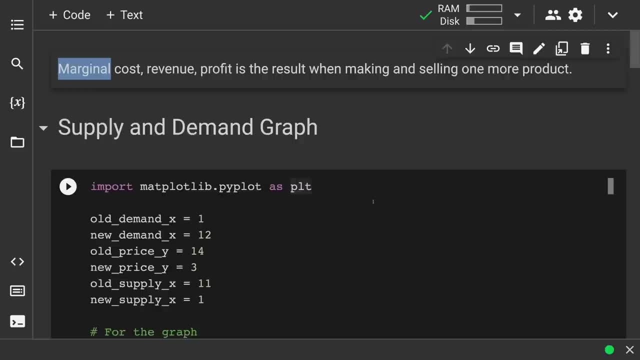 cost revenue, What's the cost of the product? What's the cost of the revenue or profit? to make one more, All right, And let's look at some other things that impact that supply and demand. And here again I'm going to give some simple numbers and make it linear equations. the 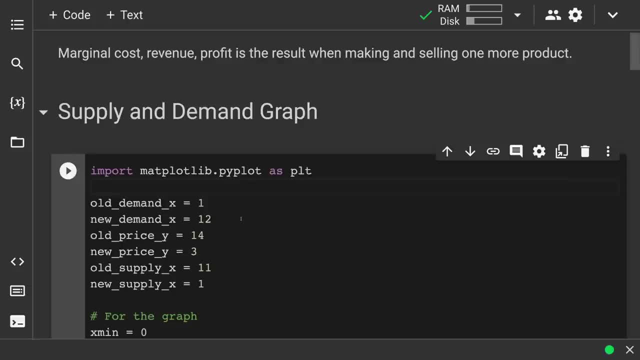 true supply and demand graph. It's not going to, you know, and in real life it's not going to be perfectly linear. Um, there might even be a little curve to it, but even at that, it you know, if you. 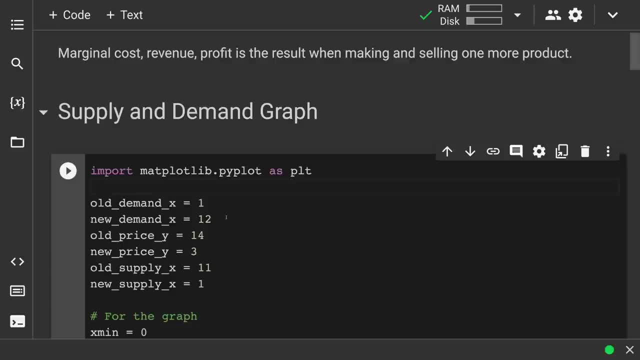 get the data. it might be, you know, a little bit of a bumpy line, But we have supply and demand and we know these definitions are. at supply, How much are people making? You know what's the supply of whatever I'm looking for, and the demand, how much will do people want? 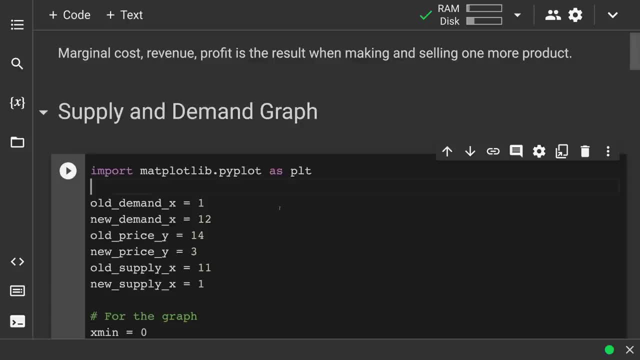 How much are people willing to buy. So you know, if you're looking at, uh, um, you know a movie, the movie theater, um, if you wanted to see it in the theater, the suppliers. there's only so many seats, you know. 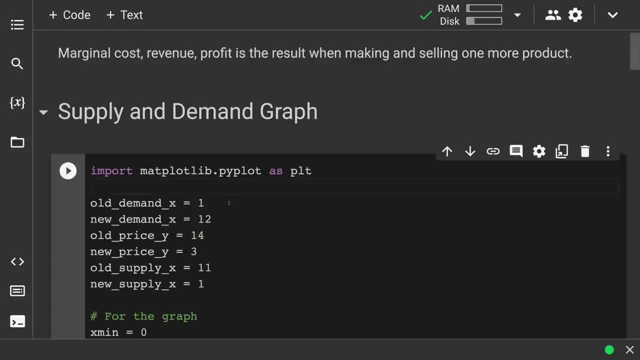 many showings. you know, a movie or a play or a concert, only so many seats, only so many showings. So that's this limited supply, And then the demand could increase if it's something really good that everybody wants to see. So, um, a lot of times we see that you know that affects. 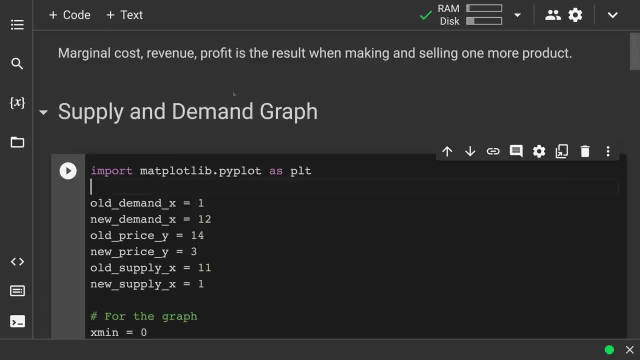 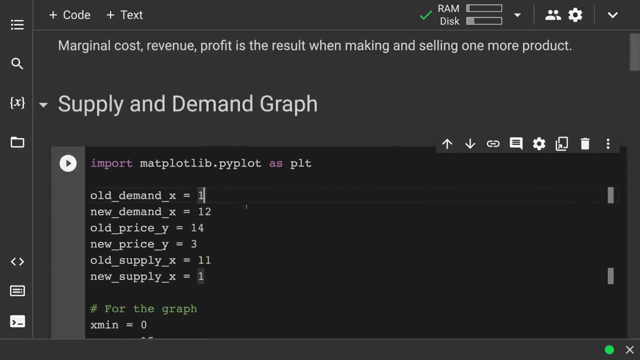 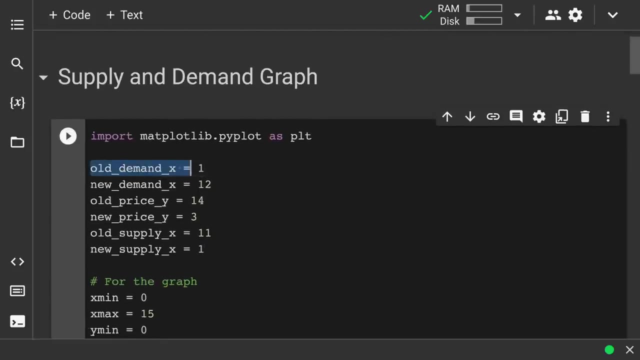 the price and that's what we're going to look at: supply, demand and price- And we're going to graph supply and demand on the same axis. So you see some similarities, some familiar things here for the graph, And I'm going to have two X values as old demand and new demand, And I just 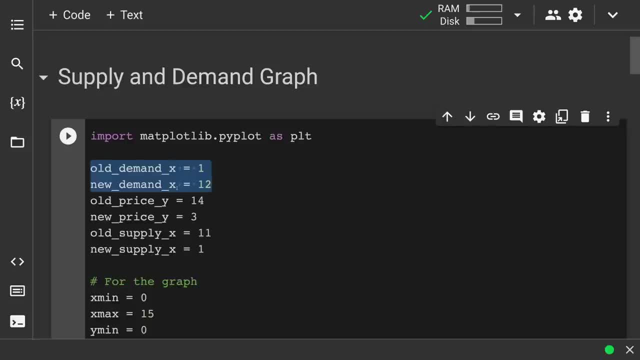 gave them this complicated variable name so that it reminds you that it's an X value. So we have old demand and new demand- And yes, I noticed I made uh, the demand um increase Um, and then I have old price and new. 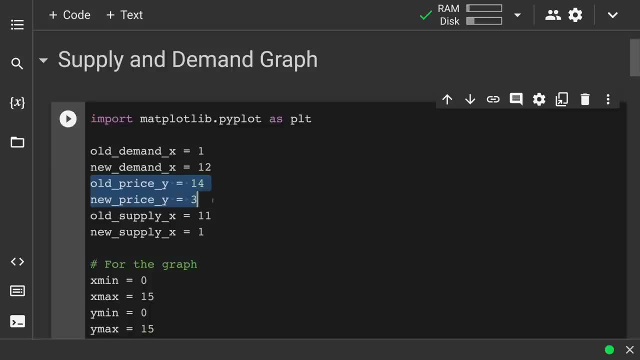 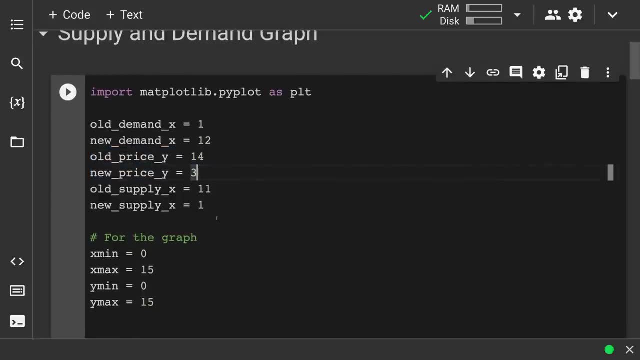 supply. So now, just looking at that, we'll. we'll see this on the graph, but the price is also going to be the Y value, And on the same graph I'm going to have supply, old supply and new supply. I made that, you know. 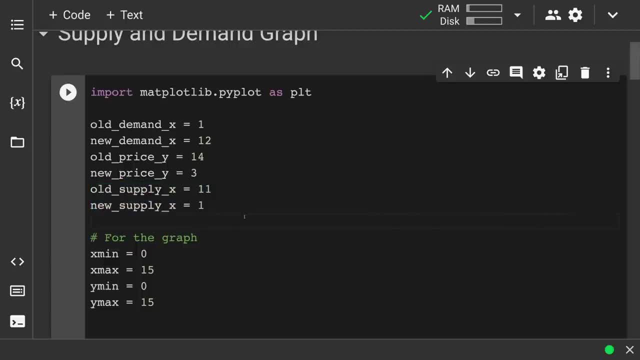 two variables Each of these. as I was mentioning, you could potentially get data from a table um- supply and demand data, um. You could have one table that has, you know, a particular price- supply, demand price- and you know, make all these numpy. 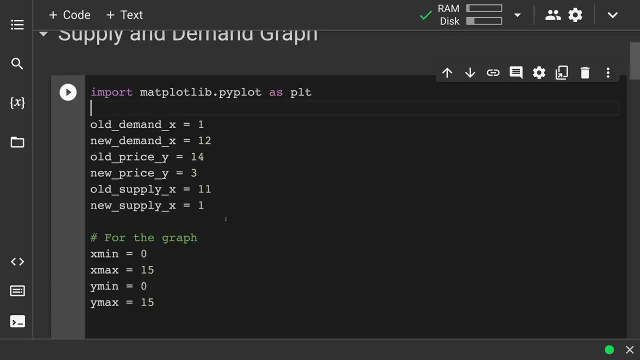 Notice, I did not import numpy for anything. I'm just putting a few variables here and you know, to illustrate the graph. But you could absolutely get data from a table and you know, make each of these numpy arrays and graph them. 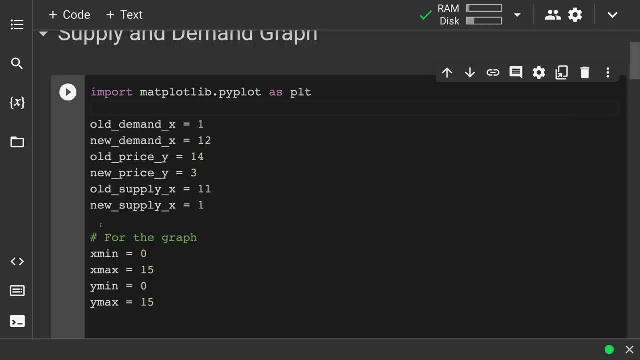 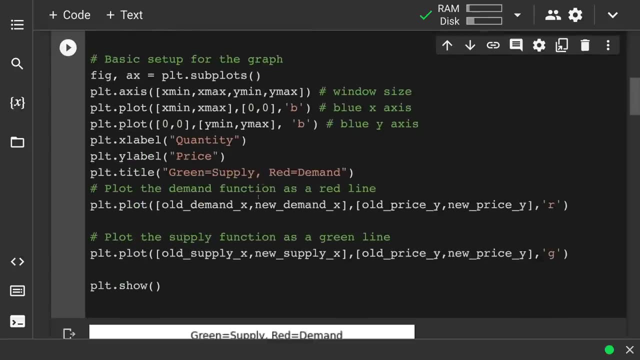 That would be really interesting too, And that's something that we'll address later on in the course. So, given these, and then I have a basic graph set up adding a couple labels here, I'm going to make the x label quantity just general quantity and the y label price. 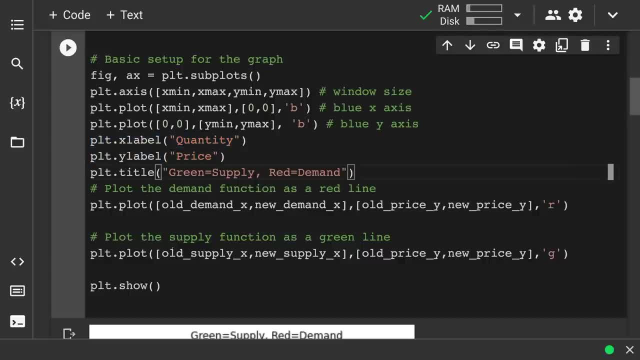 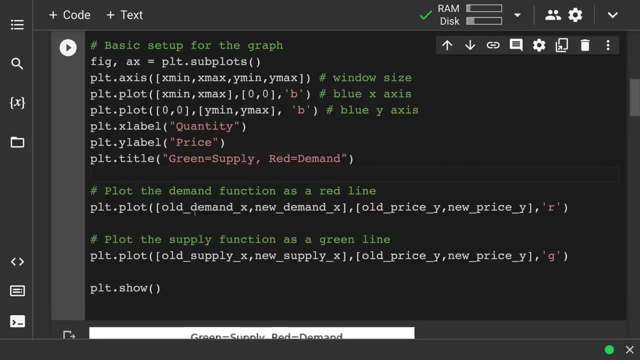 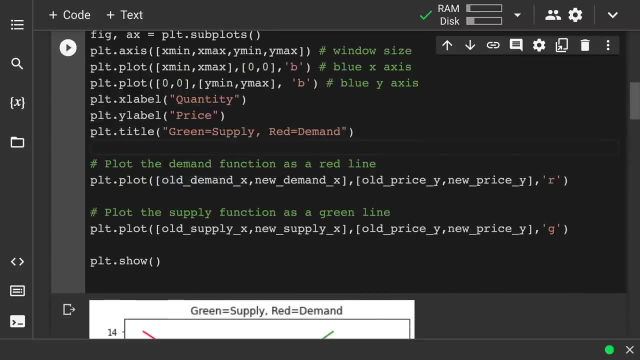 And I have this title which I already graphed. but we'll get to that. So here's the demand function and I'm going to plot this as a red line, just because. All right. so notice the x and y, my old x. I'm just making this just like I do it with the axis. 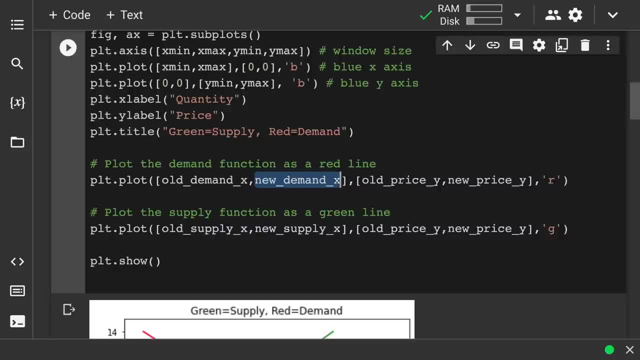 I'm going to plot, you know, these two x values and these two y values and make you know, make that a red line. So we see this, you know, I'm not going to even put an equation to it. 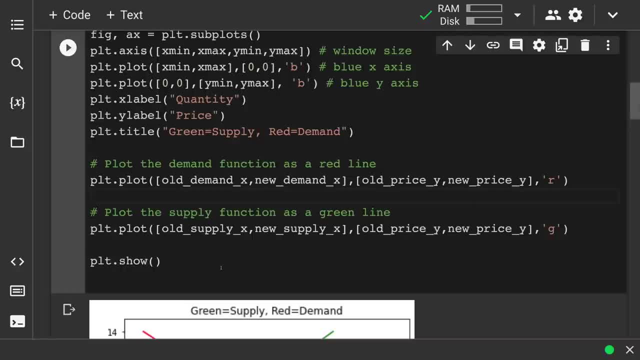 I'm just graphing this linear equation from these points to this point And I'm going to do the same thing for supply As a green line, and same thing. I'm just going to use this data that I had, these numbers that I came up with, as an example. 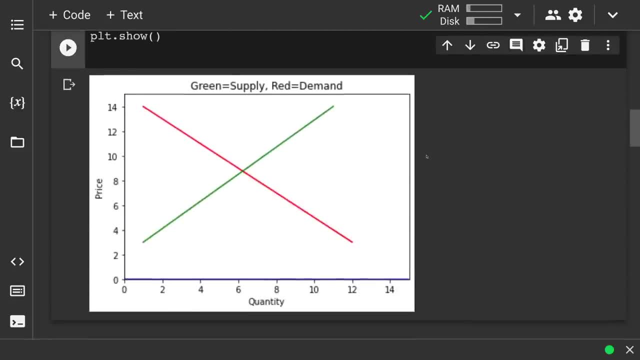 And this graph. we can take a look at this Again. it's simplified but it really is the general trend of supply and demand. So if I made green supply, red demand, then we take a look at the x axis is quantity. 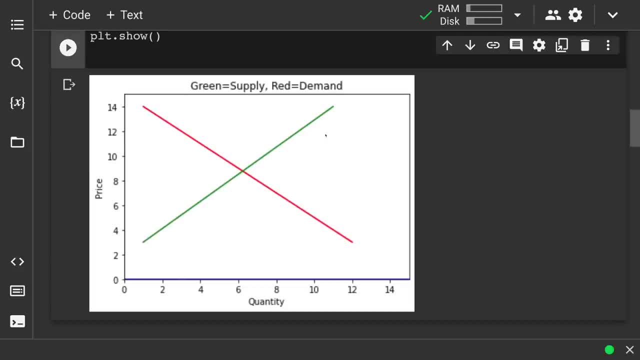 So the green, that would be quantity supplied, And the red that would be quantity demanded. And then on the y axis we have price. So graphing them both on price, we take a look at this and we see if the price is high. 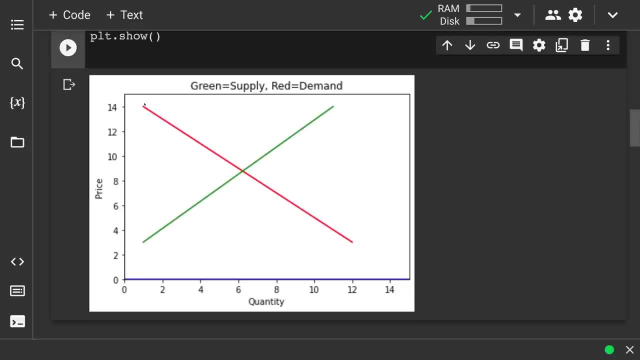 then the quantity demanded is going to be low. And a lot of times we're used to seeing, you know, an independent variable on the x-axis and we think cause and effect. But this is really correlations. So I'm not saying necessarily one causes the other, But you know it goes together. 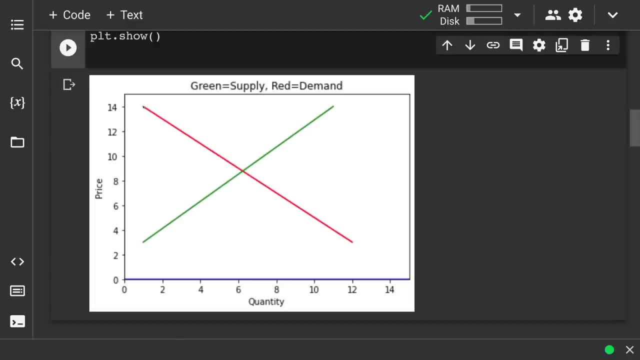 So when x is, let's say, 1 and y is 14, so we look at this demand. there's very low quantity of demand when the price is high And then as the quantity see, we see the quantity increase as the price decreases. So that's what happens. Oh, you know. 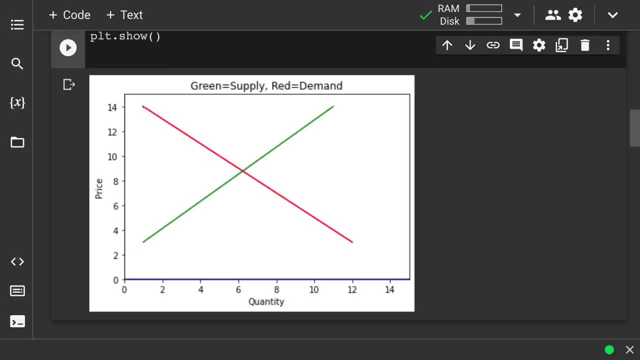 what is this? Oh, it's 14,, you know, $14.. No, I don't think I want it, But as the price gets down lower then maybe, you know, the demand increases. more people would want this Now. 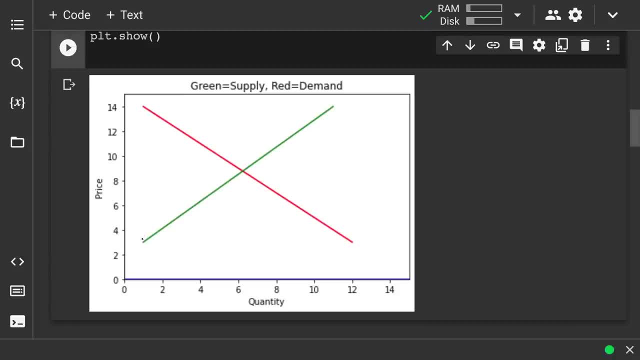 supply-wise people making this. they have a different incentive, They want to make money. So when the demand is low and when the price is low, then nobody wants to get into this. So you see we have low demand but we also have low. 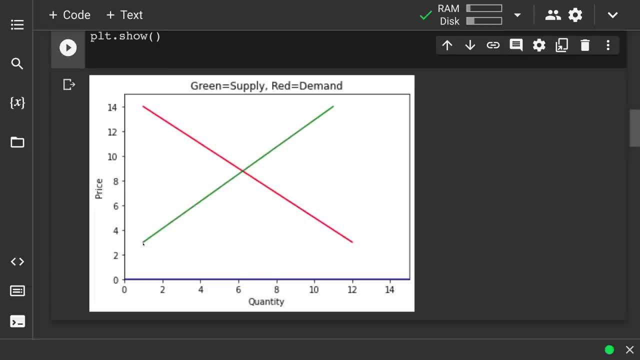 when the price is low here, then nobody wants to get into this. Why, you know, why would I get into this new business if I'm? you know, whatever I'm selling is not going to be, you know that, lucrative. But the quantity in the green line, the quantity. 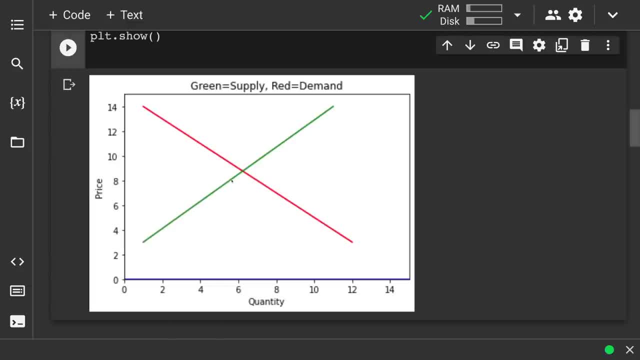 supplied will increase As the price increases, And we see that in different industries that you know. oh, you know why. why are people, you know, getting into this industry? Oh, because they all see that they can make money. Oh, this, this is the hot item. Oh, I can get in on this and somehow, you know. 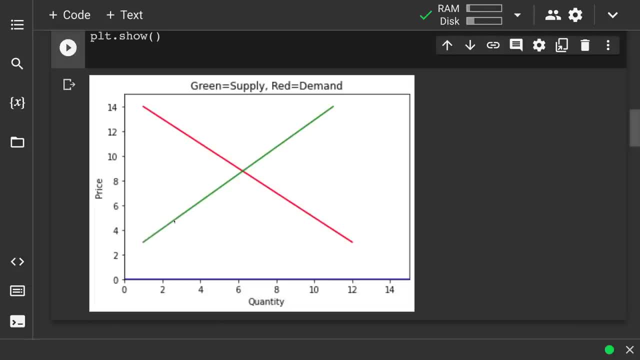 make money. So that's what we have, that the supply quantity increases as the price increases. So there we go. So we have these two opposite trends And this is kind of like the core of economics, because, as you know, I get different data. this is I just did these numbers as an example, But these 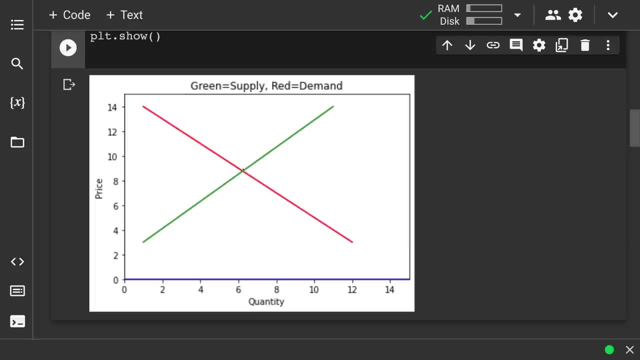 graphs could shift. you know, maybe there's some something else that affects this that maybe you know, instead of the supply increasing like this, maybe something causes it to increase a little bit steeper. or maybe you know, if we say that, you know the quantity supplied is low here for this price. 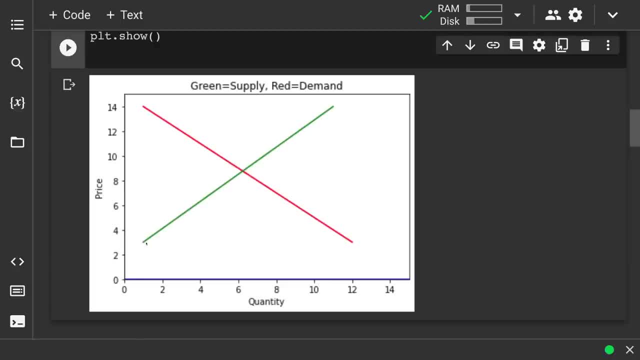 but maybe you know, for whatever we're making, that the entry level was even at a higher price and this whole thing shifts. so you know that's really what a lot of economists are trying to do. and then, if this is quantity across the x-axis, let's take a look at where these lines intersect and then 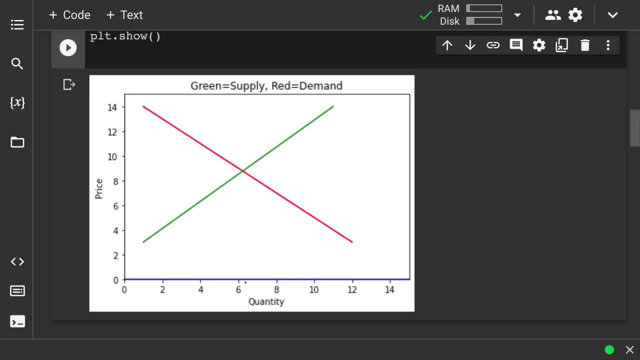 that would be the point of equilibrium, because what we're saying is the quantity here supplied and the quantity demanded would be the same, and i mean that's ideal, you know? um, you know, let's say you have a bakery, you make fresh things every morning and then at the end of the day you have 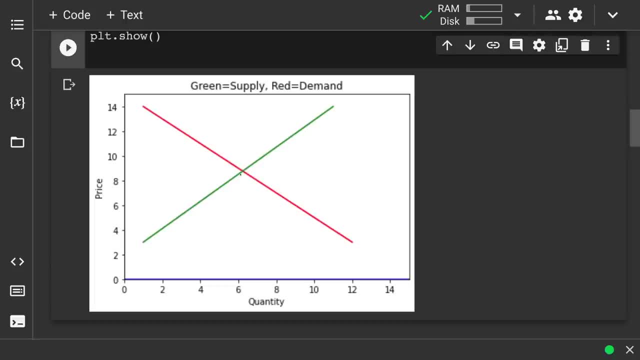 it all sold, nothing left over. that's great. um, here on the left, you know, and we'll say, let's say that you know, you know, you know, for our fictional numbers that happens at six, but let's say a little bit before that. so it's still. 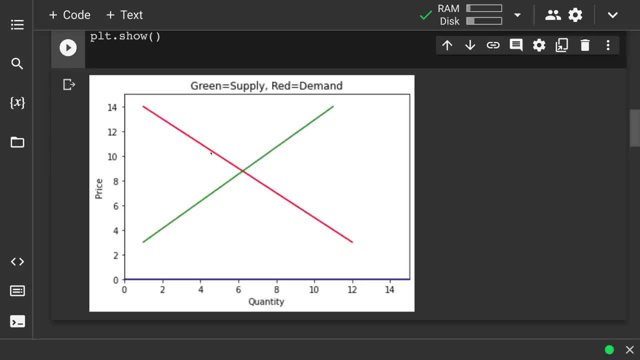 to the point that the price is too high, so the demand's not really there. the price is increasing, but not so good yet, so the supply is not really there and we still have a gap between demand and supply. so here on the left the red line's higher. there's more of a demand, but not enough of a 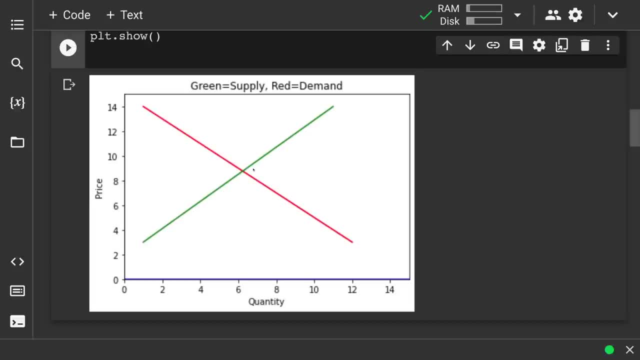 supply, and then we have on the right side of that, we have more of a supply but not as much demand, and that would be the one- this would be on the right. that'd be the one that's dangerous for anybody supplying whatever product, because you know they're getting into this trying to make. 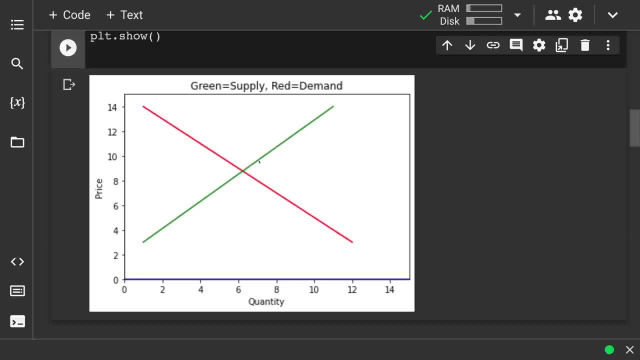 money. the price is starting to get to where somebody's happy- oh god, i'm going to have to. the price is going up, i'll make more money. but then there's, you know, the demand drops off. so now they really have to scramble for customers. you know that's trouble: or the price here or on the. 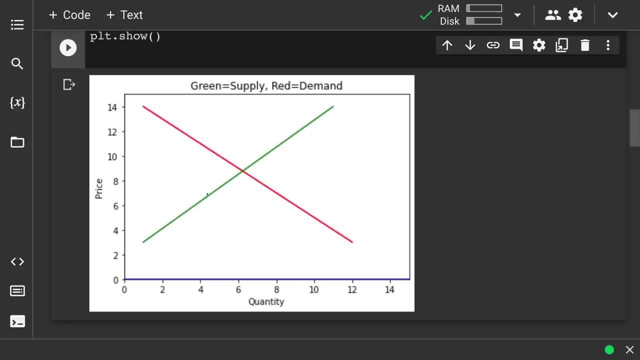 left for the people who want this product. the demand is still higher than supply, and that's part of what keeps the price higher, because the demand is there, not as much supply. well then, the people argue about this stuff all day, anytime somebody wants to. too many people want to sell. 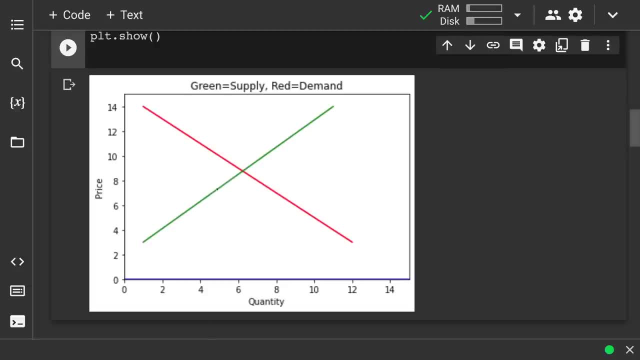 a particular stock. oh well, then, you know, the supply increases too many and we go to the right. too many people want to sell this. um, you know, then other people notice that turn- oh, you're really trying to get rid of this, and then the demand kind of goes down. you know what's wrong? 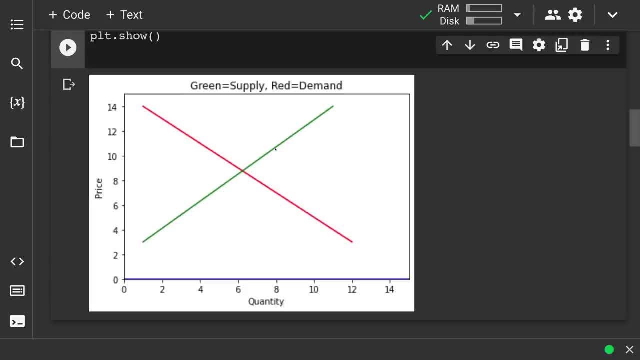 with it, um, and that affects price. and on the left then we have: the price is too high because there's not enough of supply. supply and you know that sometimes causes, um, oh there's, you know there's not much supply. nobody wants to sell that you know this must be good. and then that kind of increases the demand and the hype a little bit. 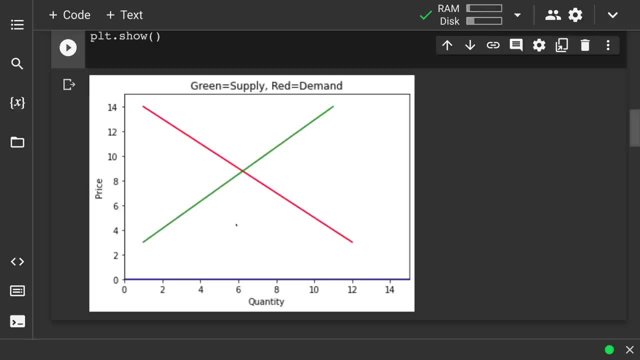 so you see, this one simple graph describes all these complicated trends and we see this that you know. our goal all around is, you know, finding these points of equilibrium. supply meets demand. you know. therefore, everybody, you know, making whatever products are making money. people looking for these products are finding them. you know, and you know fair trade: people are paying reasonable. 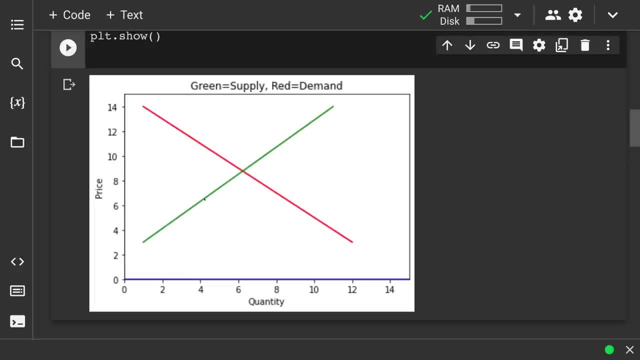 prices. we're all trying to get to that, but we see all these things happen all around there, and it's not just one direction of cause and effect. it's multiple things going on as well, as it's not just one direction of cause and effect. it's multiple things going on as well. 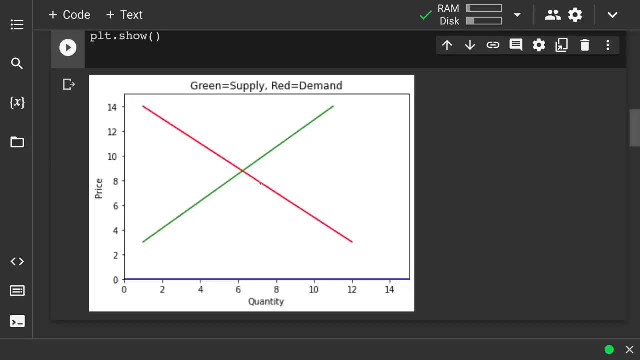 as just general correlations, all things happening together. so we look at this, you know, and, and let's say we say the trend is like: as the price goes down, how does how does that affect demand? or it goes the other way too: as the price goes up, how does that affect demand? 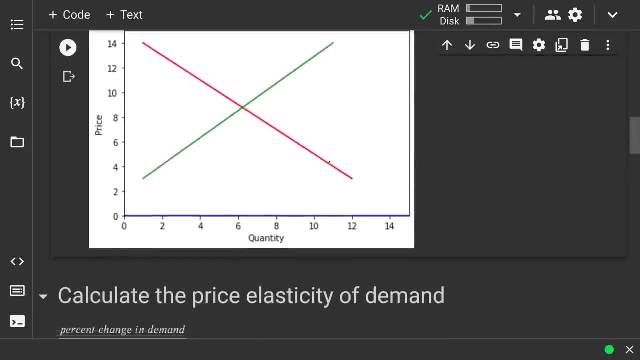 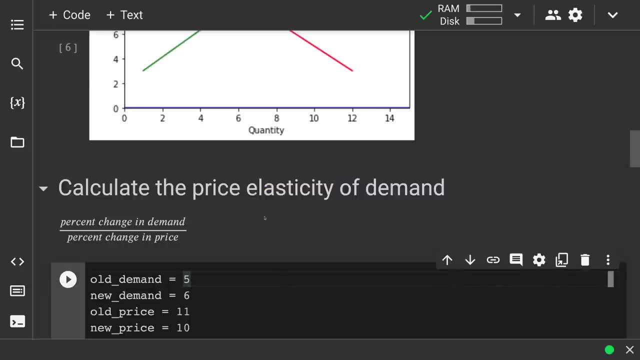 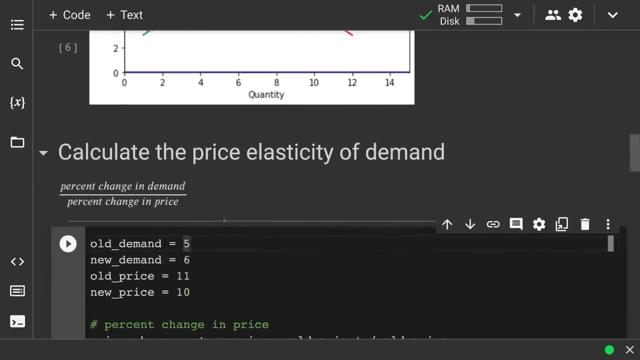 and the word to describe that is elasticity. so elasticity is: how quickly does demand change when price changes? and we can look at this. there's the formula percent change in demand over percent change in price, and this is again all these economic formulas. i'm just going to give you a couple of them here that when you have these formulas, you can use this. 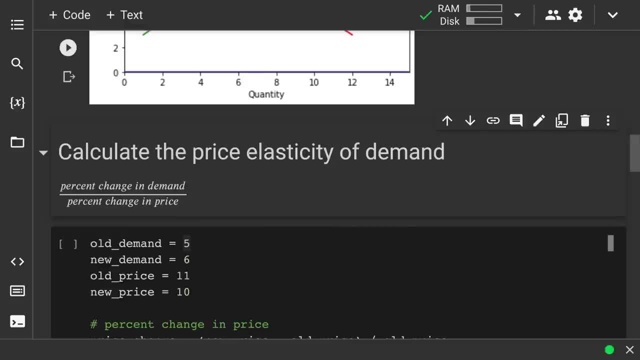 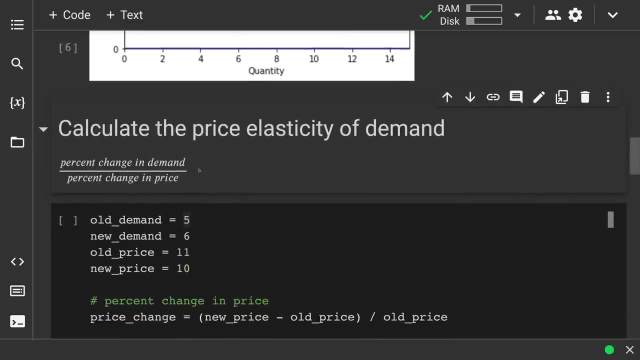 you know, get data, use it to graph and then use it to calculate these formulas, to answer these questions. you know how elastic is this? the difficulty on that side of the equation, and then to broker the, is that price, because if things change, if the price changes, and then that. 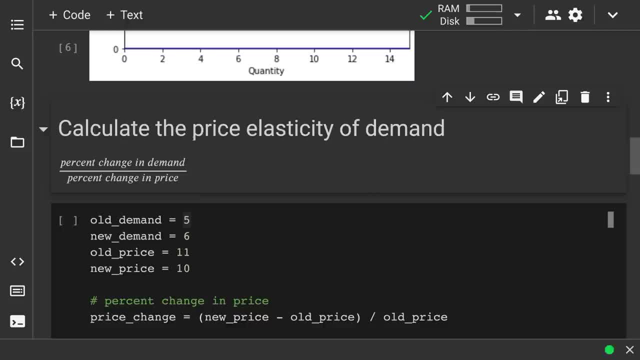 really changes demand, then we can say it's a very elastic like it, like an elastic band or something that bounces, that you know it stretches and changes easily or things you know. if price changes and it does not change demand, you know things like gasoline, yeah, we don't like to pay, price goes up, we don't. 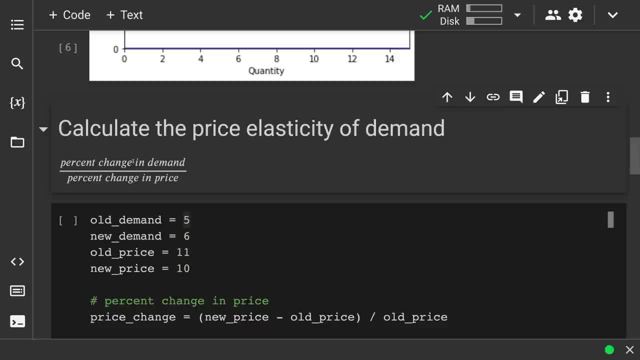 like to pay it. but if the price went up a little bit, I still have to fill my car, so that demand would not be very elastic. the price could change and the demand doesn't change and you know we can, so we can see that if the percent change in. 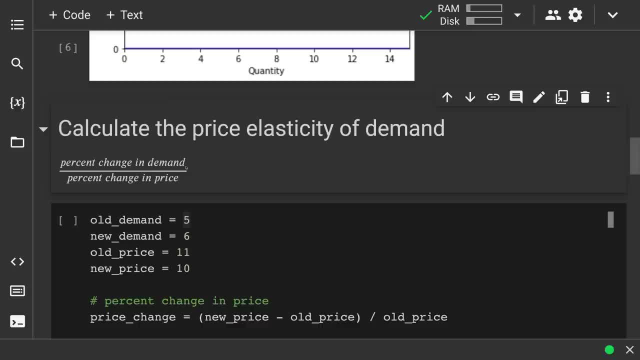 price. let's say it's, it's you know some significant number, but then the percent change in demand is like almost nothing. we calculate that you know the total value of that fraction is going to be close to zero and we say that's not very elastic. but maybe some other things you 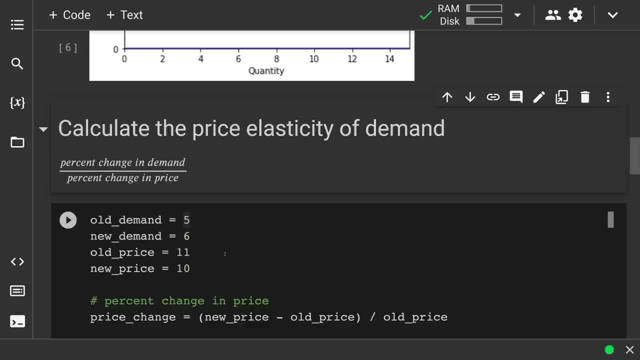 know a concert ticket. you know there's ones. I've seen where. oh, I'd like to go see. I'd like to go see this, but the price is too much. no, I won't go. and as the price goes down? oh, I heard the price went down. that would absolutely change. 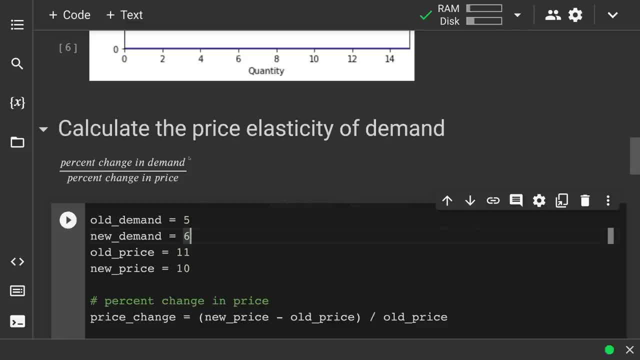 the demand. that would change the price. that would change the demand. that would change the price. that would change the demand. oh, too much, I won't go. oh, the price went down, now I want to go, and that really changed it. you know things that aren't essential and we would say that that would be very elastic. so in 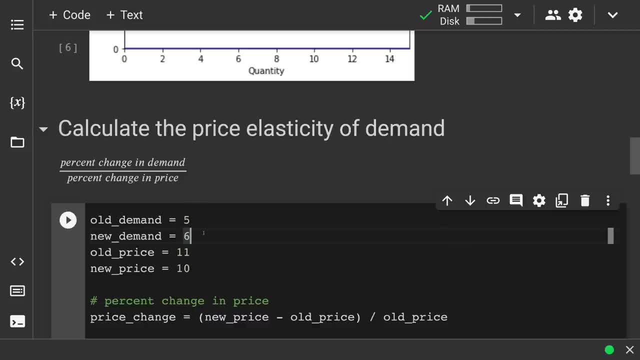 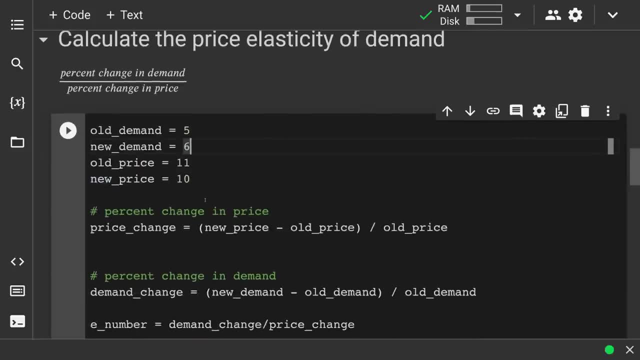 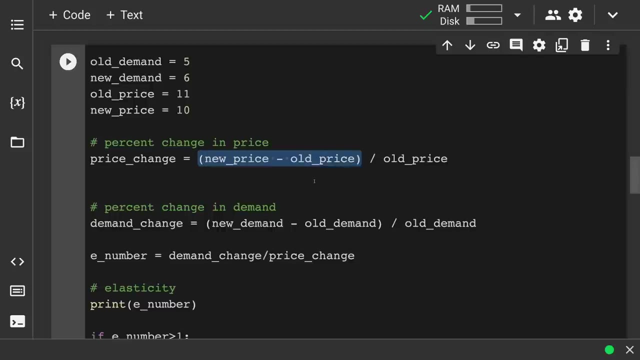 calculating this, and you know, down the road you could always combine all these into one thing, but I'm just gonna show you, like just, old demand, new demand, old price, new price, and we're gonna calculate the percent change. so remember then, that's, you know, the new price minus the old. so there's their difference divided by the. 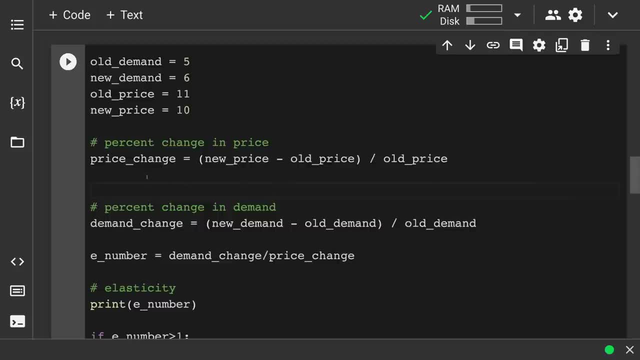 old price and it's going to get a decimal that we can convert to a percent. so you see again, and we want to get in the habit, like you you're so familiar with. you know collab that. oh, I have a formula I want to use. you know write. 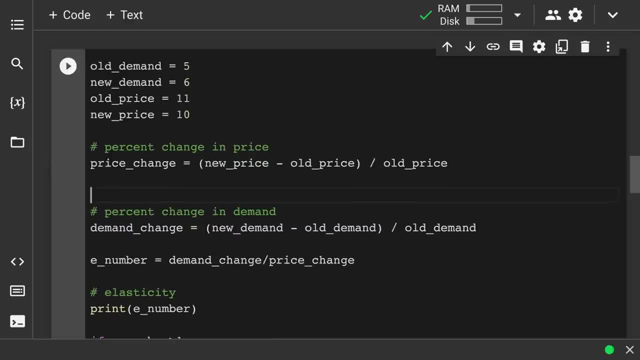 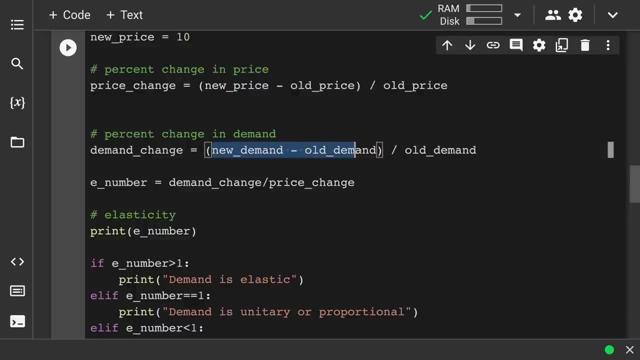 write a quick program to do it, and then now all we have to do is change these values up here and we can calculate everything that we need. so price change And that ends up being the percent change. And then the same thing with demand: The new demand minus the old demand. 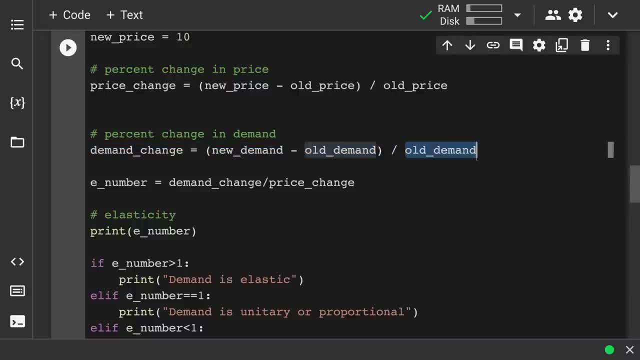 And that's the difference divided by the old demand, And that gives you a percent. It will give you a decimal that you can convert to a percent. And so elasticity number is demand change divided by price change. So what I have is: then it will just print that number. 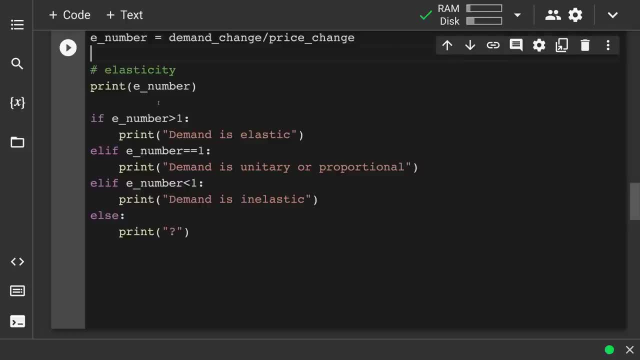 And here's some of the analysis. So again, different things. Oh, what's the cutoff point? You can always just put these in a nice little if statement, And so if the number is greater than one, then I'm going to print: the demand is elastic. 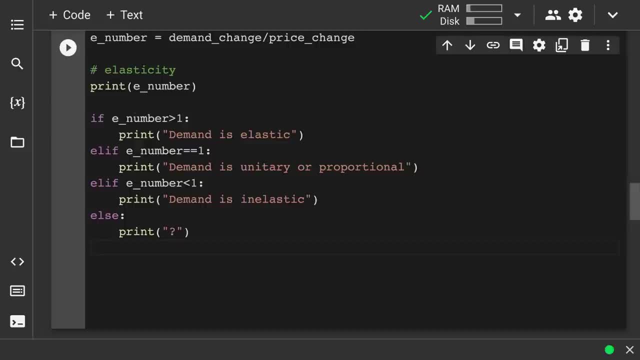 And notice this is else. if So I just continue this on. You know, elif number equals one, Then It's unitary or proportional. So sometimes you know we do get one. that's there you go: An increase. I think that proportional increase increases demand. 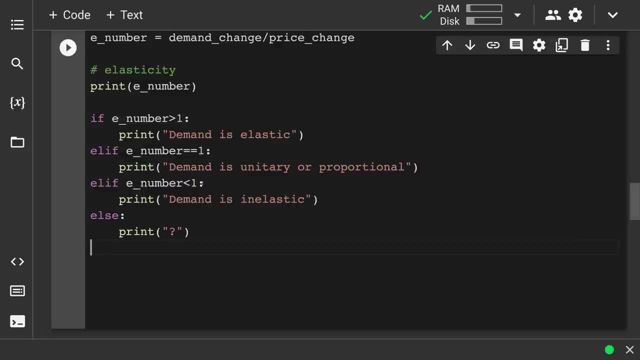 But you know, And then if it's less than one, then that's any elastic, That's. those are all the ones that you know. again, it the demand hardly changes based on price. And I just decided to tack one more. 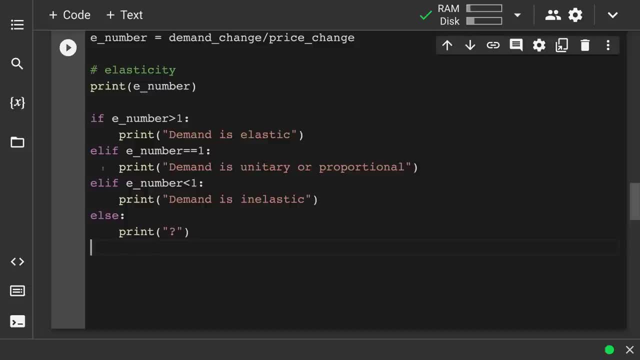 And so you see, this is how you can. You know, I like to when I do my elif statements. I like to tack on one more thing at the end. you know, for whatever reason, you know, this should capture everything. if it's either greater than one equals one or less than one. 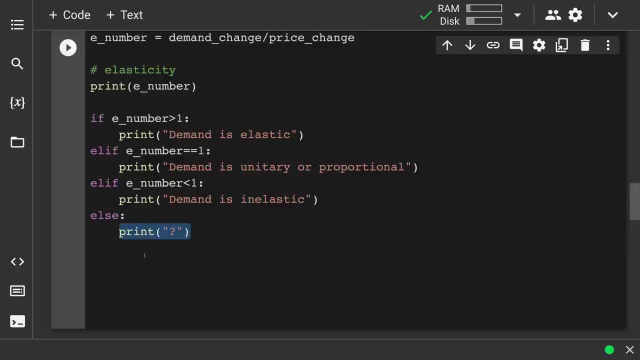 I mean it's really but capture one of the like grab bag. you know what. you know if something else happened, very often will have if an elif, without you know, exhausting every possibility, And then you just easily Just put an else there at the end. 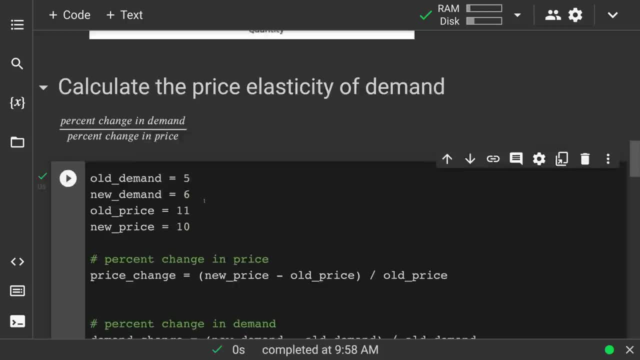 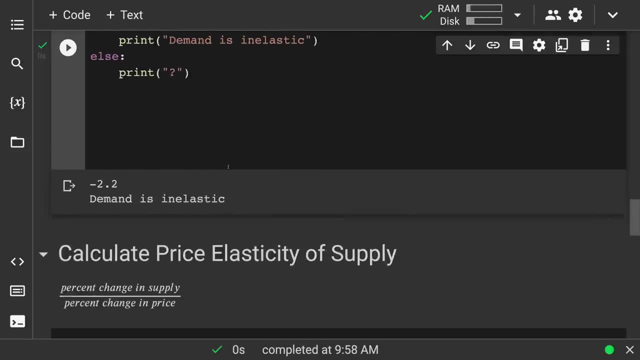 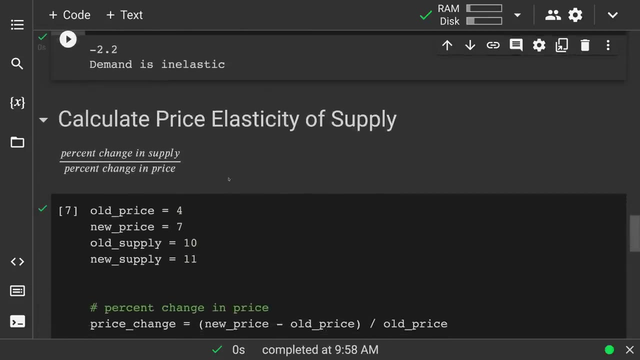 So I have some sample numbers here and then we can click and it would print out. So we get this negative two point two and then demand is inelastic. So as that example, And we can do the same thing with supply. So remember, you know, supply changes as price change because people say, oh hey, I want it. 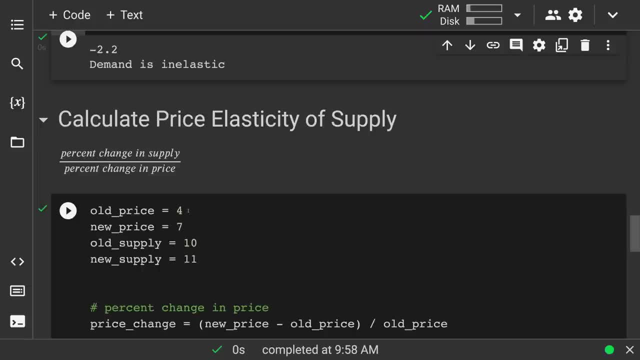 This is, This is a hot industry, I want to get into this. or then people say, oh no, it's. you know, this is cooled off, I'm going to get out. So in the. you know, in the United States kind of recently the real estate market was hot and that supply like, OK, not everybody necessarily is going to sell their house or try to be a realtor or try to sell some property. 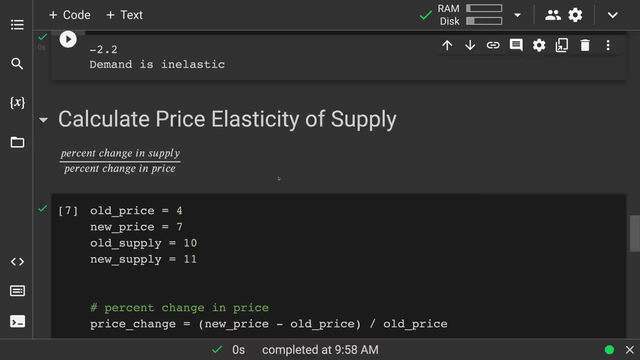 But when the prices are so good, More people decide to get into it, like, oh, maybe I will sell this, you know. so that's the idea that if the price is good and people see, oh, opportunities to make money, they get into that. 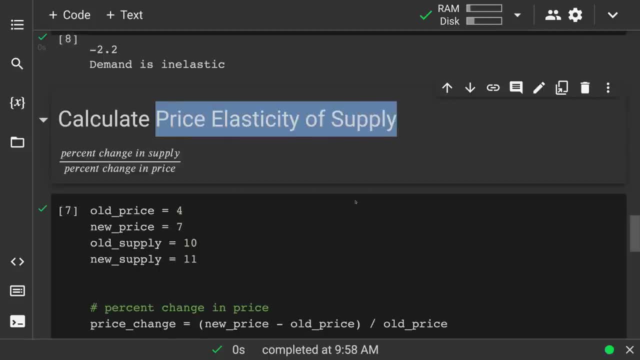 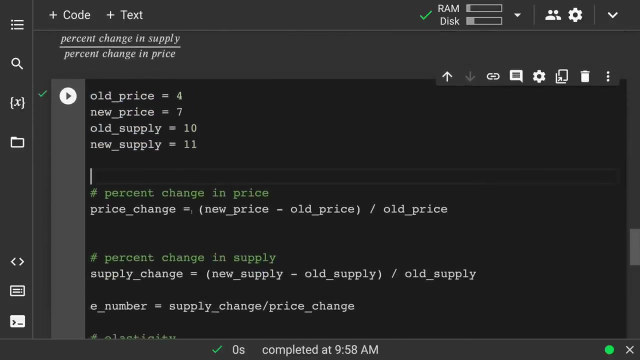 So price elasticity of supply Answers that question: how, How responsive is this supply To changes in price? So very similar formula: percent change in supply Overprice, Percent change in price And just a few values to Sample. and very similar formula. 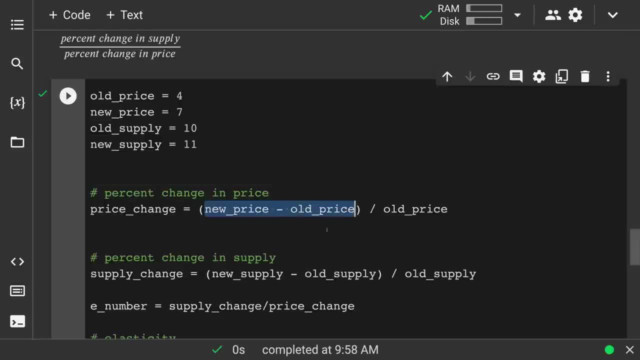 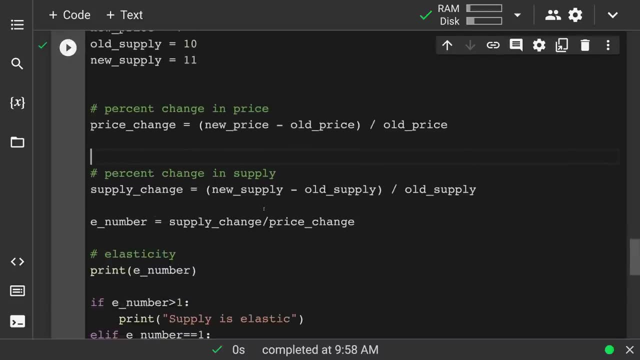 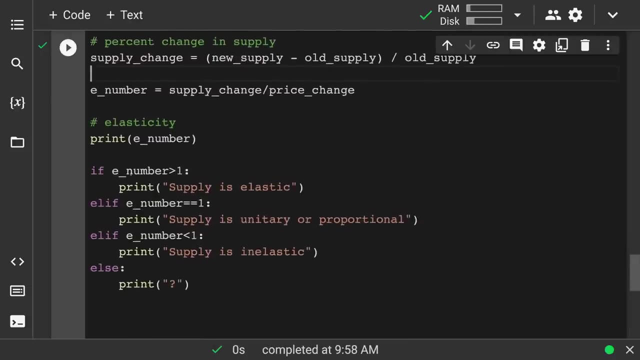 You know, new price minus the old price divided by the old price, and New supply minus old supply divided by the old supply, And we're going to go through the same thing: Elasticity, number and Very similar analysis: greater than one It's. 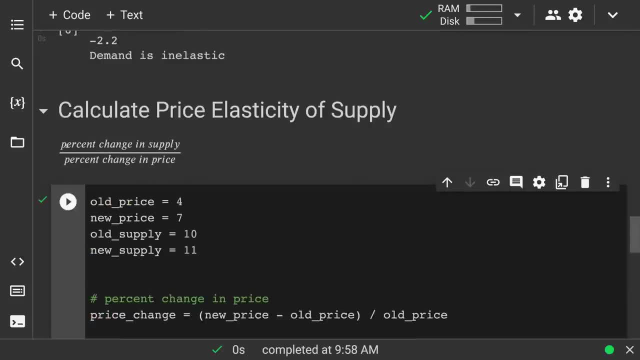 Elastic, which remember, as a fraction greater than one, is going to be that this percent change in supply is much greater than the change in price, percent change in price. and we have to do percent change because if we just do, you know actual dollar amounts or actual number of things supplied. that really doesn't always give us a good example. 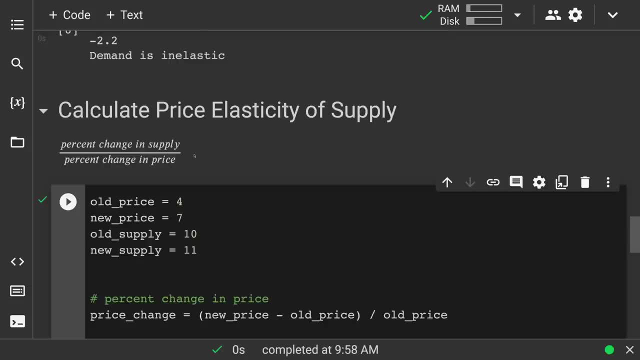 Some things, just in general, are low cost. So a change of a dollar might be a whole lot. Some things are really high cost, like you know. a change for a car, that price change of a dollar is not going to be much at all. 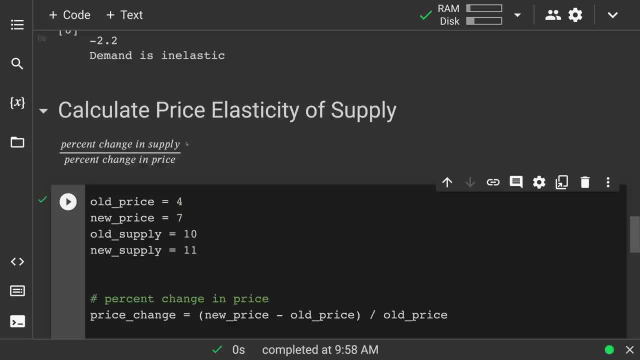 So same thing with supply. you know what, what's, what's the relevance, You know how is it relevant to the previous supply. So that's why we do the percent change. So yeah, if price changes, You know a certain percent. 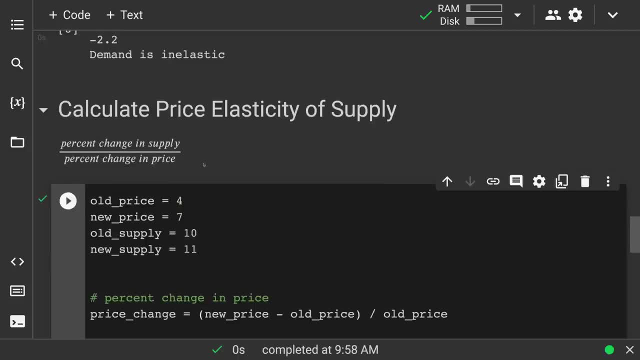 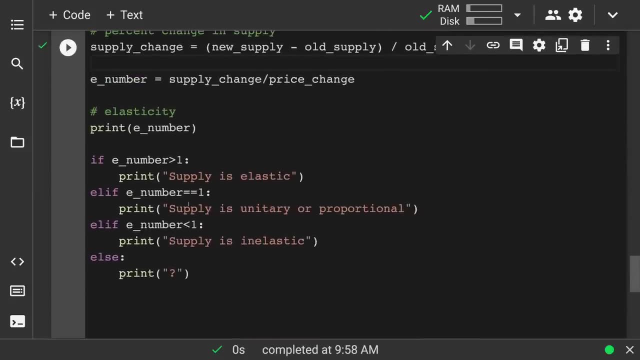 But supply changes a lot more related to that. then we're going to say, oh well, that's elastic. People are noticing these trends And we can go through this and same exact analysis: either supplies elastic, unitary or any elastic. 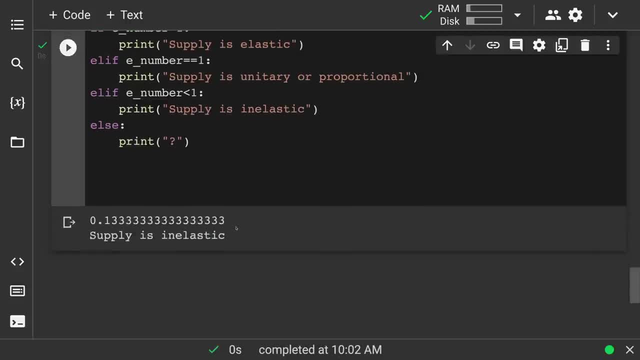 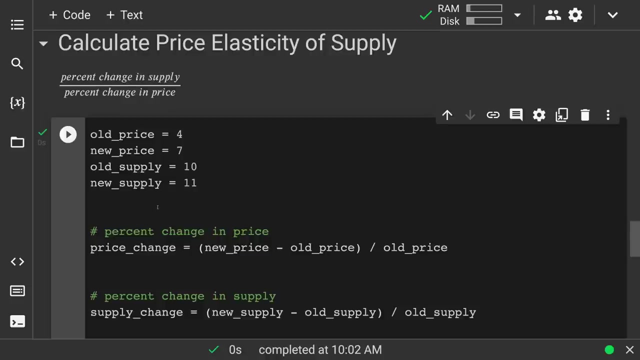 And you know, just had these. So there we go, This number, and it's inelastic because it's this tiny decimal. So, yeah, not everything you know. supply cannot always be, you know, elastic. And so, notice, you can take this and, given the old prices and old supply, you could always take these things and combine them with something like this: 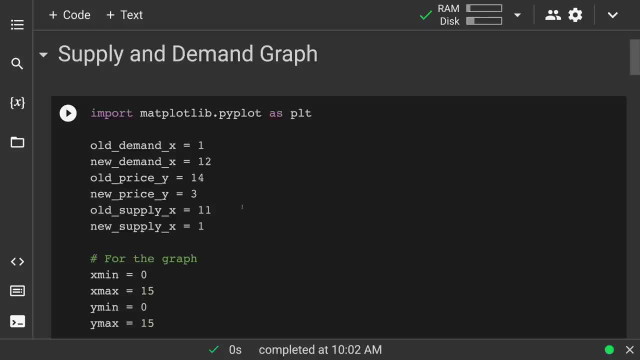 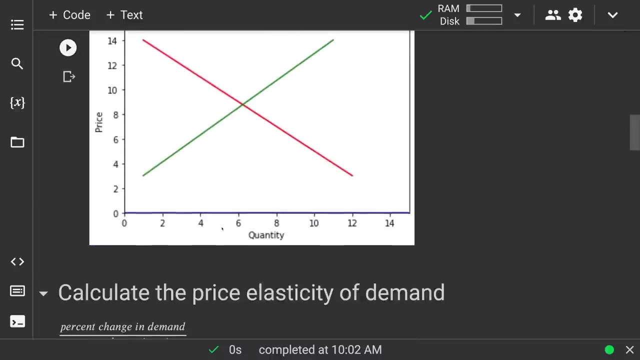 So, therefore, you could graph, and if you had, you know other, you know other numbers. So notice this. I mean, even though these numbers might be fictional, if you had any bit of research, that you just had a few values here, you can get these. you know, and with these you know six things: calculate, you know the graph, and elasticity of supply, elasticity of demand. 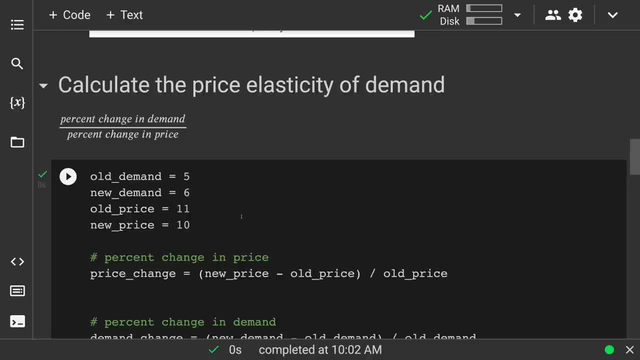 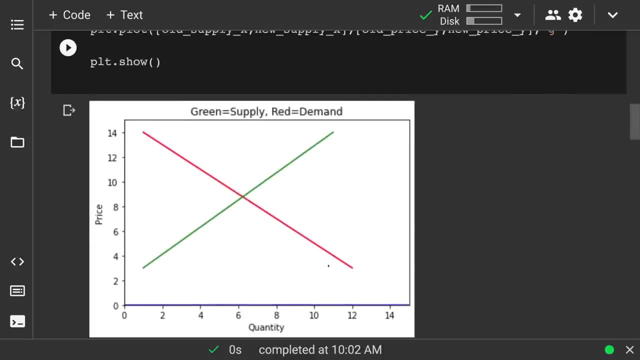 And really just get it Handle on. you know where, where you are in this graph and what are the potential changes. You know, is it? you know these graphs. I kind of made the linear and it's kind of proportional, but you know, very often it's going to be bumpier. 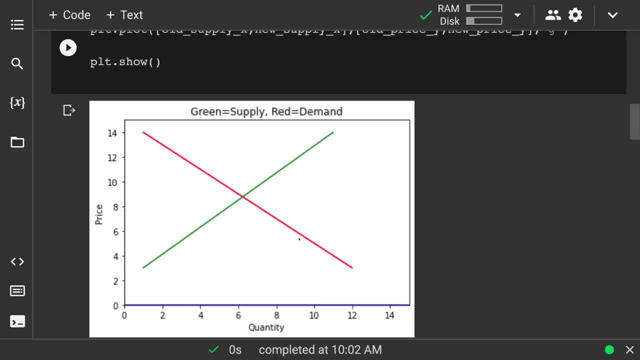 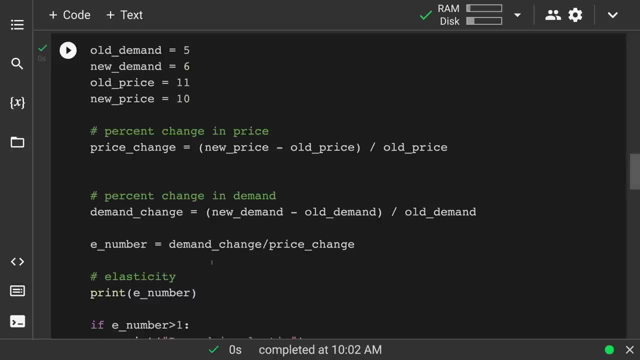 And you know where are you on this graph and what's what's what's going on. If you really wanted to, you could even there's other plugins for other Uh data, especially things like stock prices, and you could use this uh to calculate um elasticity for various stock prices. 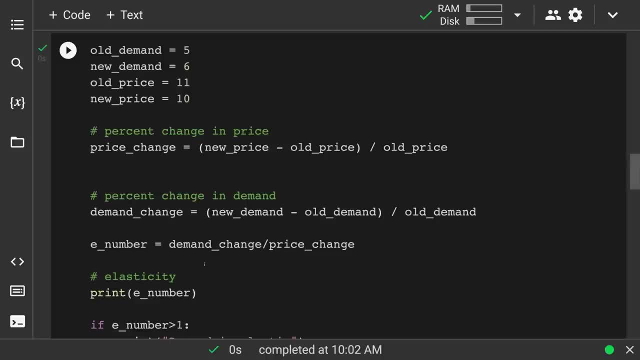 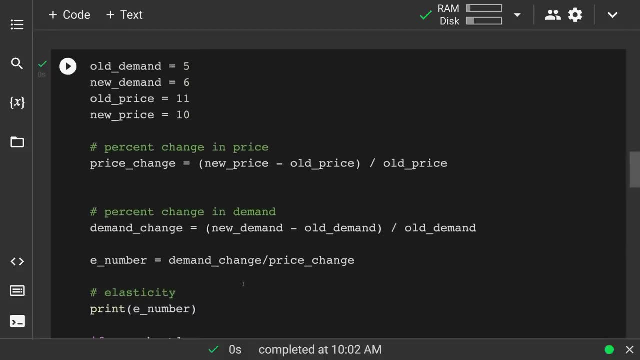 You could calculate some of the trends um, and a lot of these it'll work within Colab. There's a lot of things that'll work within Colab. There are a lot of things that'll work um within your Google drive, and those particular free tools tend to update things like stock prices. 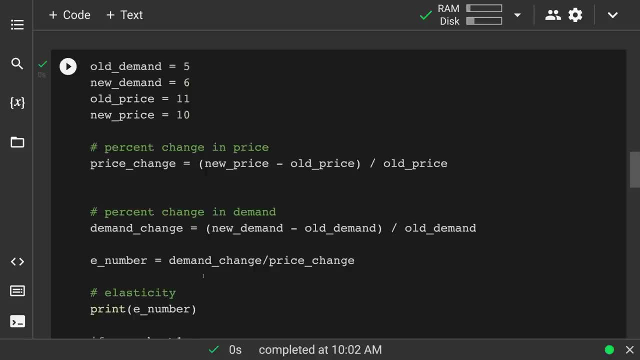 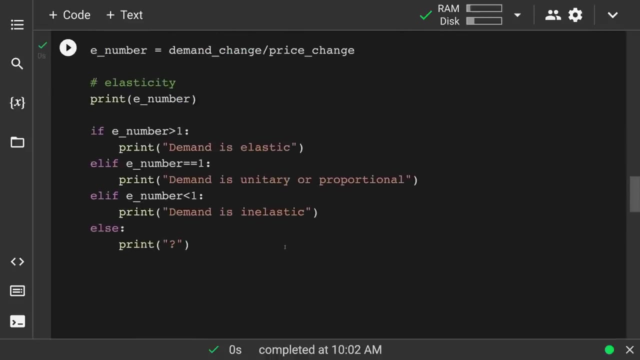 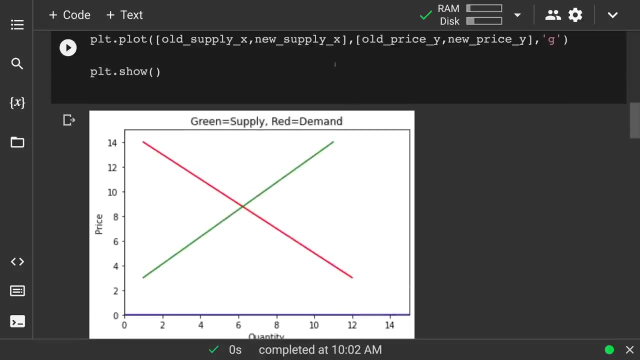 Maybe like every 15 minutes at the at the most, but that's going to be enough to give some sort of analysis, you know, for an amateur investor. take a look at different things. Um, you know, that's kind of what we want to: take this and like these types of formulas and build upon these so that you know you can, uh, build data pipelines and get information at some reasonably regular rate. 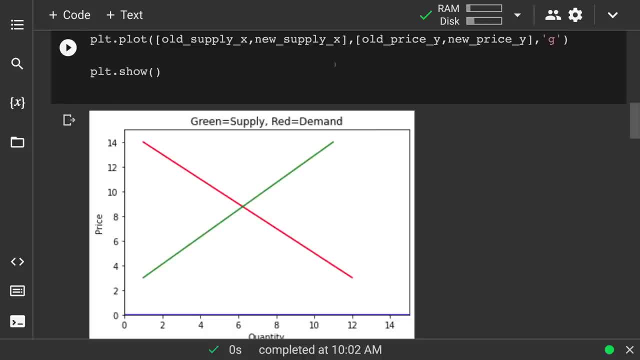 So if you're going to have a new product at a particular level, um, have all the formulas And calculate and say: you know, okay, now you know, have this output at some sort of report for you. Let's see the graph. let's see it in real time. 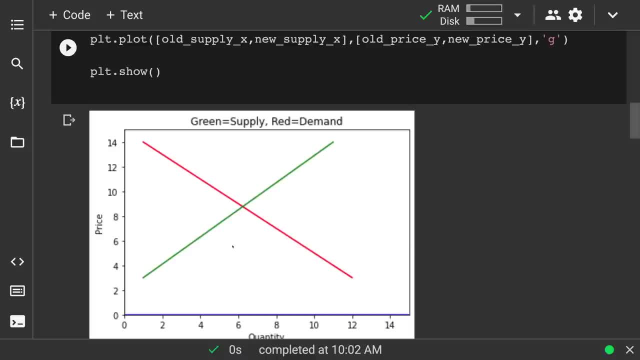 You know pretty much real time. let's run through some formulas and see you know, Hey, I'm thinking about investing in this. What, what's it looking like? Oh, it's, it's, it's very ill. You know the demand's very elastic. so you know you really have to take notice of the price. um, or oh, the the. 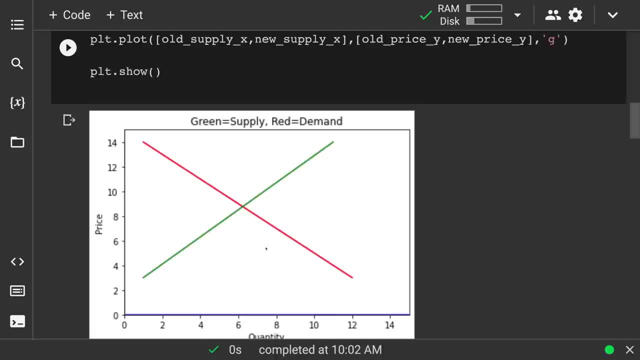 this. you know, I see this trend. maybe you know a supply of something that maybe I can get into. All these things we want to, you know, use this information to make decisions about what we want to invest in. Yeah, and you can do this all right here in CoLab and right here in your Google Drive. 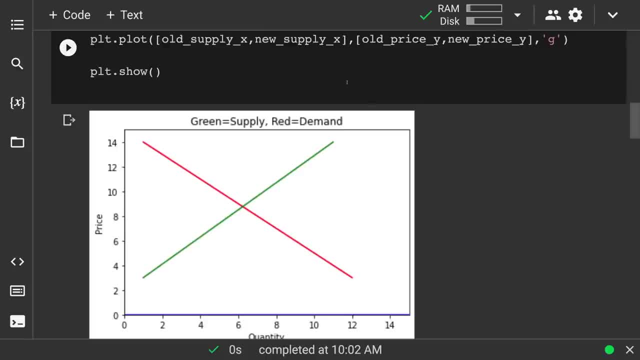 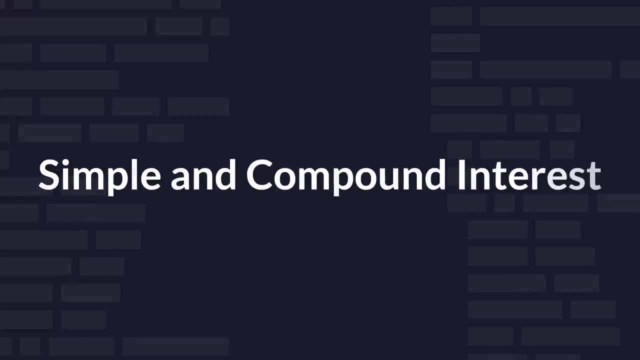 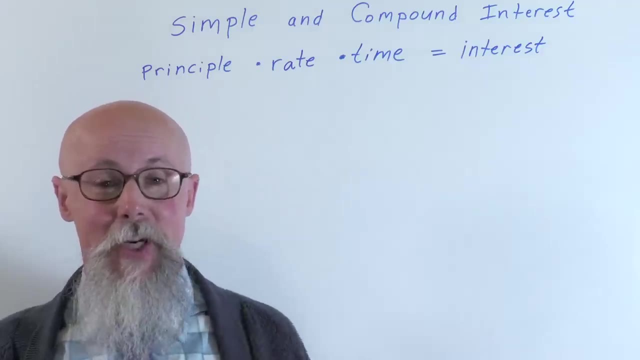 So we'll get into some more, some more math now. and you know the next step of our journey. So let's talk about calculating interest, And usually that's going to be money I put in the bank or in some investment, or sometimes it's going to be money that I borrow. And then how? 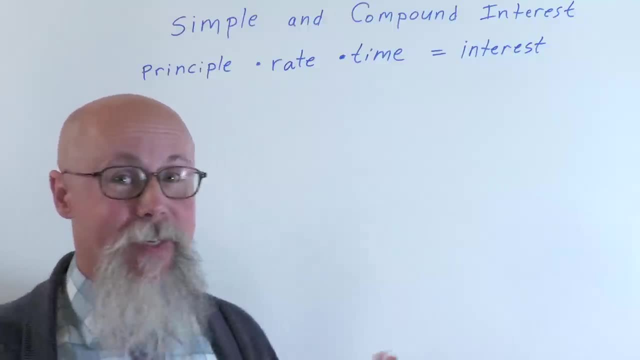 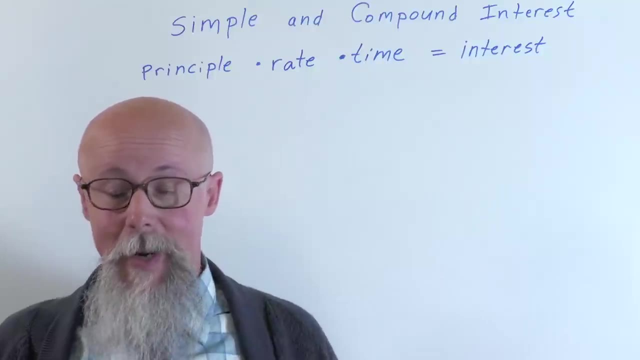 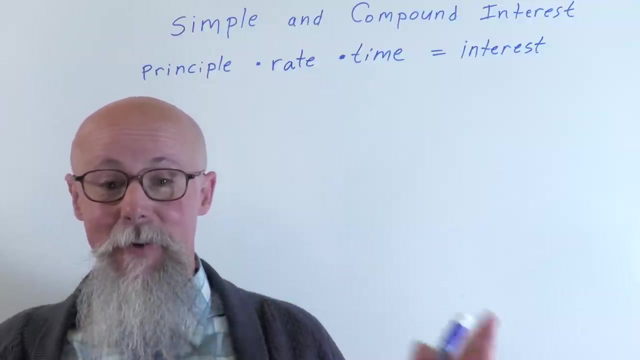 extra am I paying? So the simple interest formula is exactly that simple And it's good for short term. It's good for, you know, not a lot of money if it's long term. But the longer you go with this, the less accurate it's going to be, And we'll see why that is. But for short term. 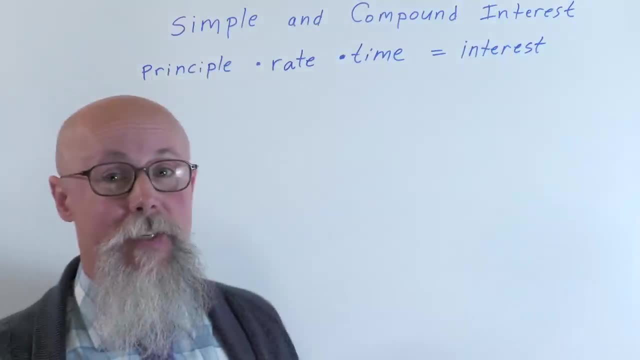 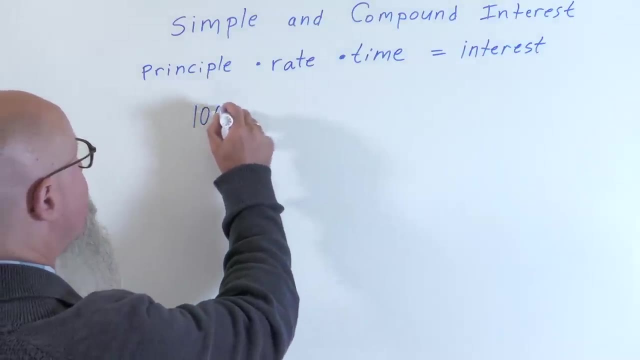 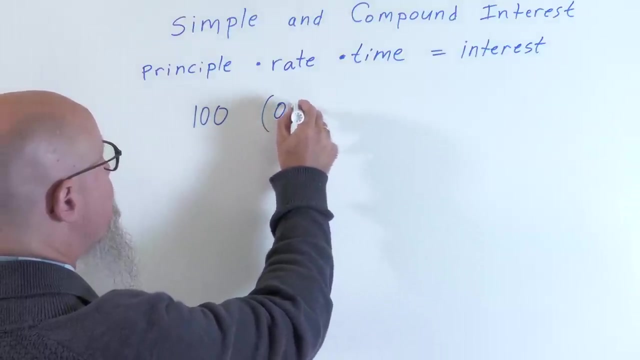 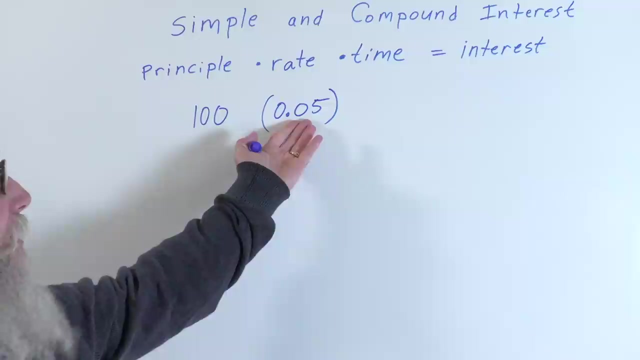 principal times rate times time- it gives you the interest. So if I was borrowing something you know- let's say you know I have borrowed, you know $100, and the rate would be 0.05.. So the rate's always a percent converted to a decimal. So the rate would be 5%. 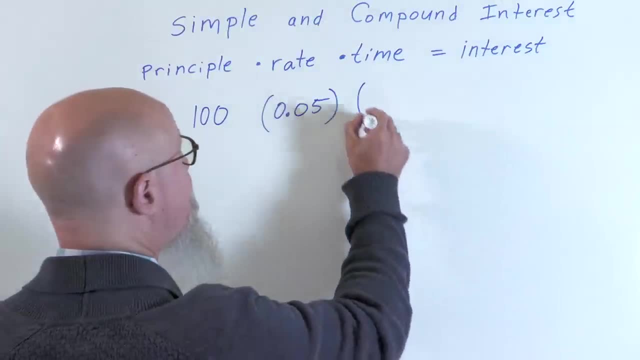 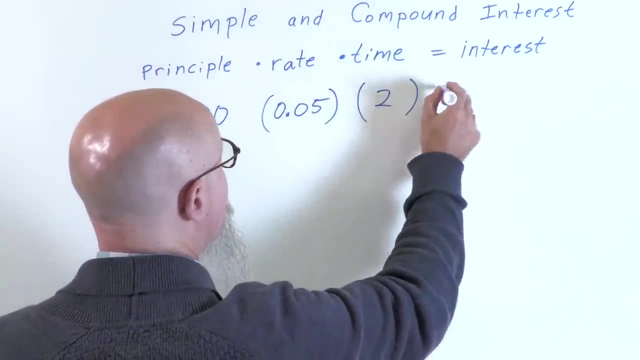 and as a decimal it'd be 0.05.. And then the time would be always in years. So you know, let's say I borrowed $100 for two years, Then what, in what extra interest, would I owe on that? 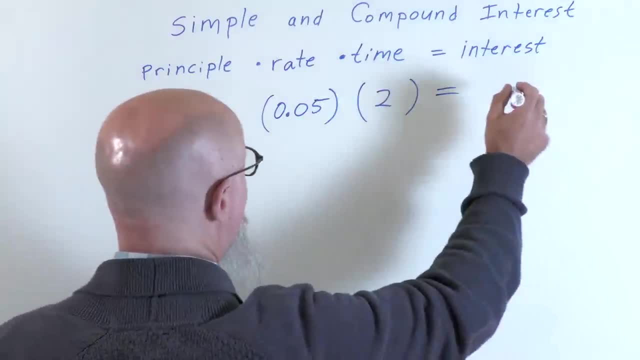 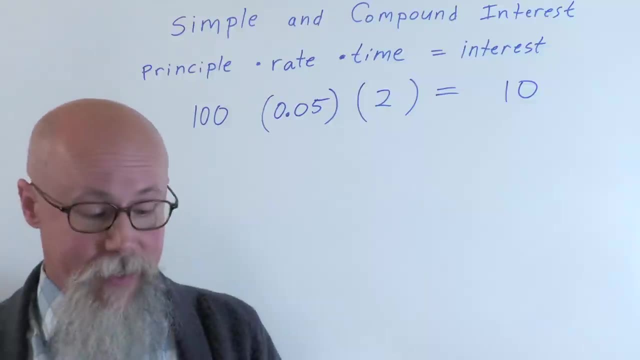 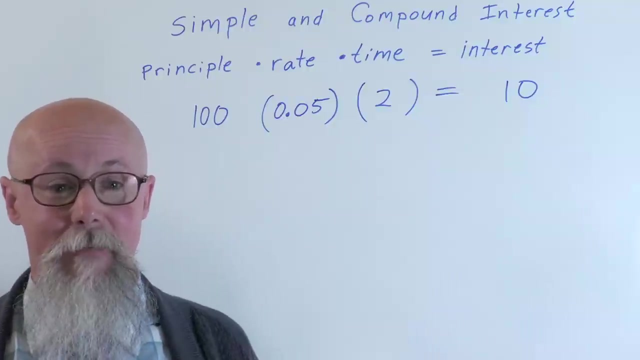 So there we go. That would be another $10.. So what I would then say is: okay, well, you know, given this rate, if I I needed $100 now and it's going to take me two years to pay it off, You know, maybe if it's going, 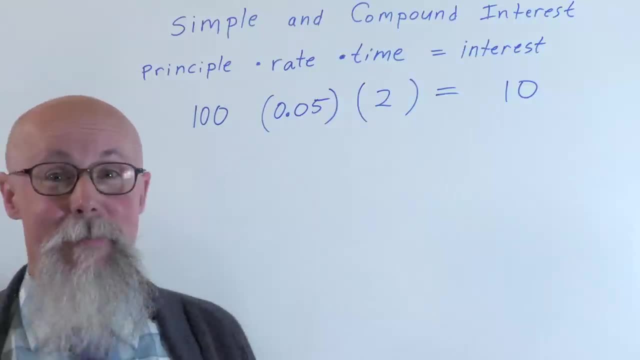 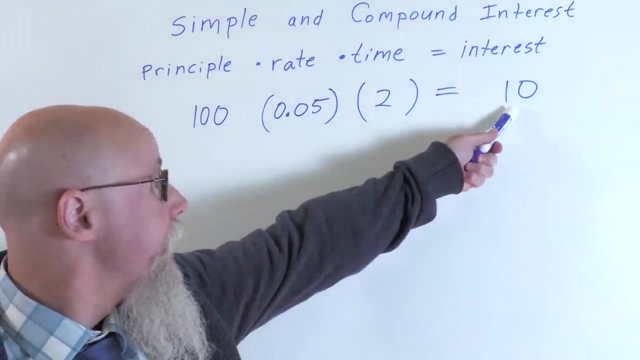 to take me two years to pay off $100,. maybe calculating interest isn't my biggest problem, But the if I, if you know I could calculate, oh, how much extra would that cost me an interest? Now, to figure out the total amount that I would pay, I would take that interest and I would add: 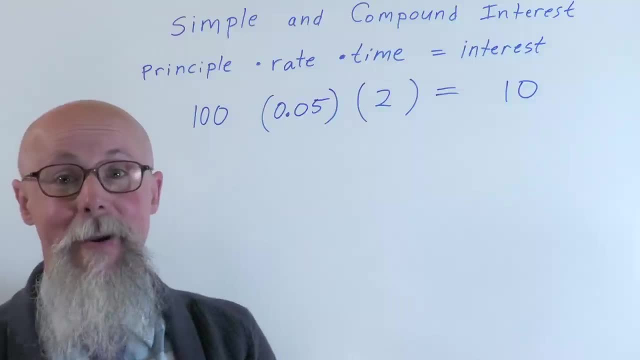 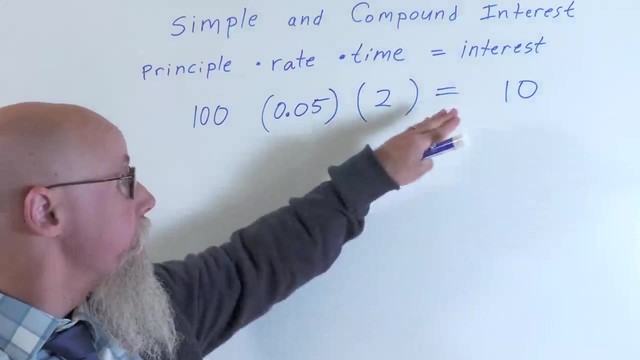 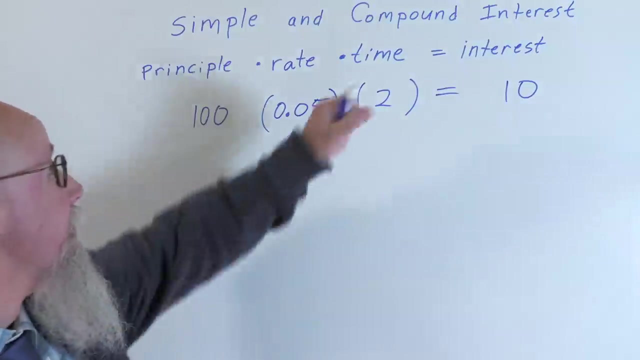 it to the original principal, because I have to pay that $100 back plus the extra $10.. So let's take a look at this. You know, if time is one like, let's say, one year, And what that is is that's compounding, That's the notion of compounding that I'm taking that interest. 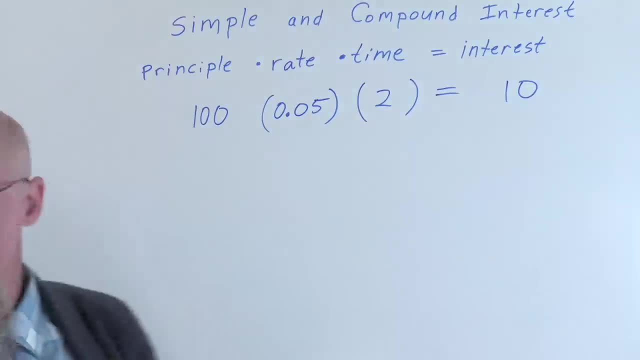 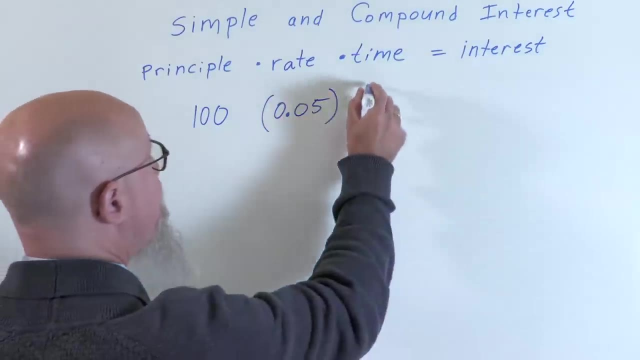 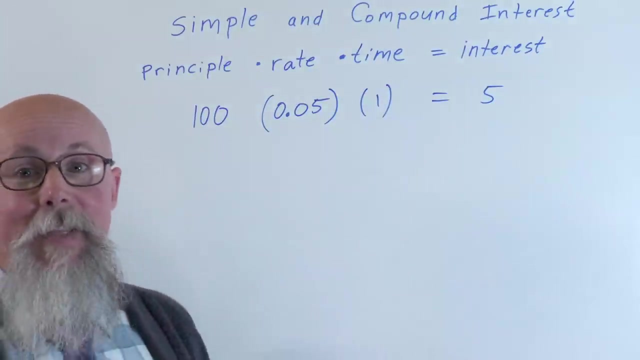 and then I'm adding it to the principal. So let's say the time was one year And so, so this would be times 0.05 times one. Then the interest would be $5. And then what am I going to do? I'm going to, I'm going to add that. 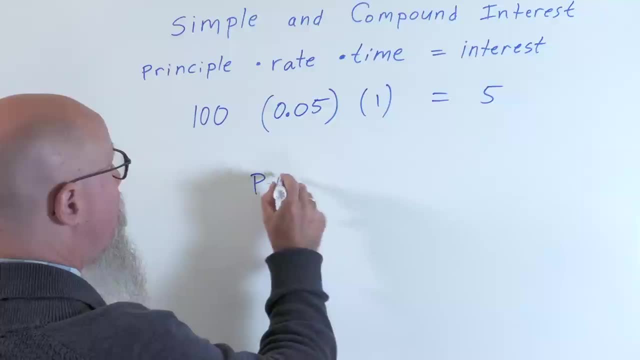 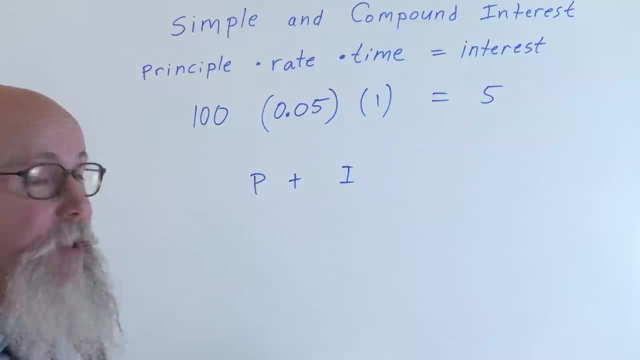 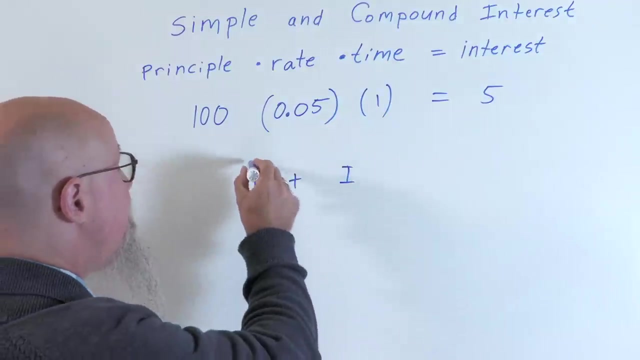 together. So I'm going to say, you know, the principal plus the interest is going to be $5.. Now the reason why we compound it is because after, let's say, a year, so then I have that new principal plus the interest, but then that new principal plus the interest, that's my new amount. 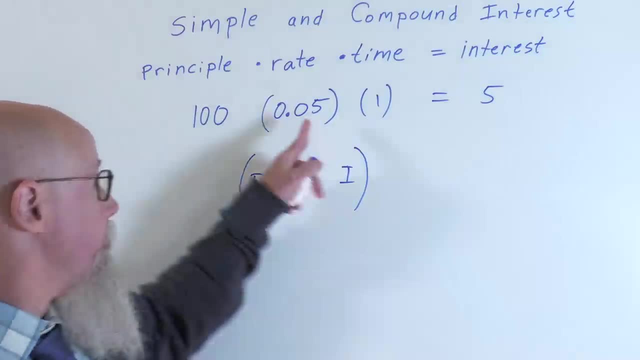 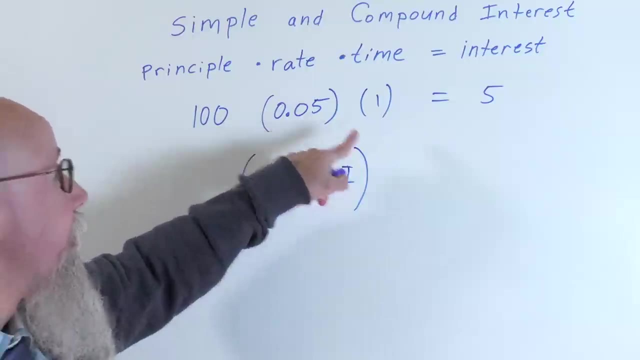 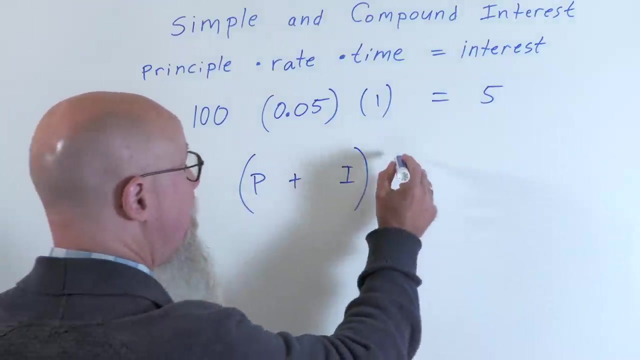 And then that would then generate another 5% in interest. So you see, that becomes my new principal. times 5% gives me my new amount of interest. And then I'd have to add that. So you see, I would take that, you know, times that 0.05.. There we go. 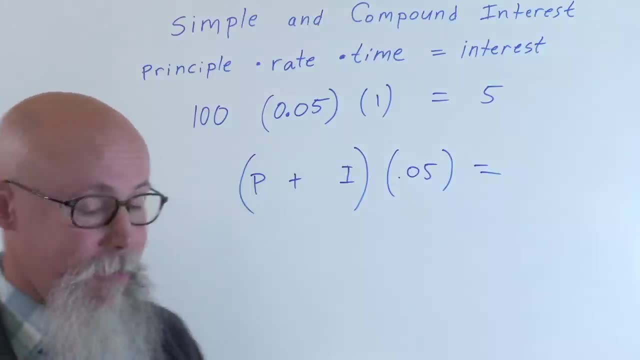 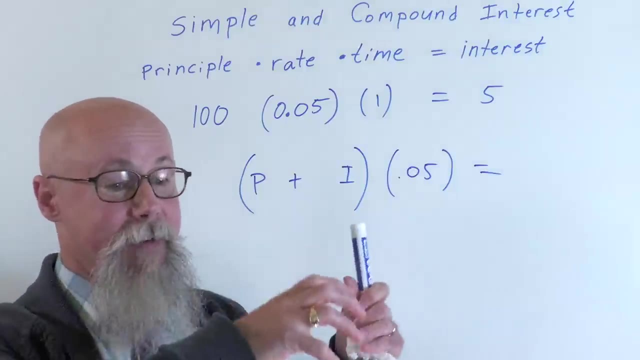 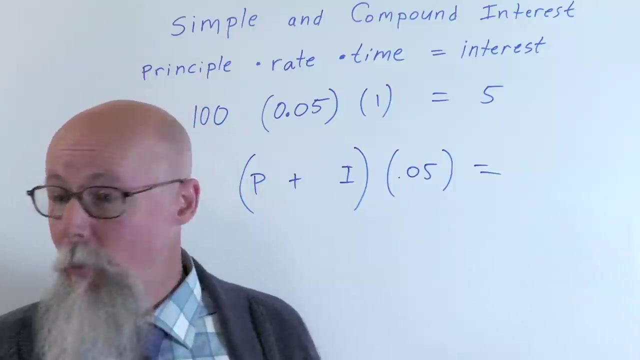 And then I take that amount and add it to the new, new bit. So that could potentially be a lot. You know, every time I have to calculate the interest, add it to the principal again and then recalculate it. But let's take a look in terms of algebra: what, what's really happening? 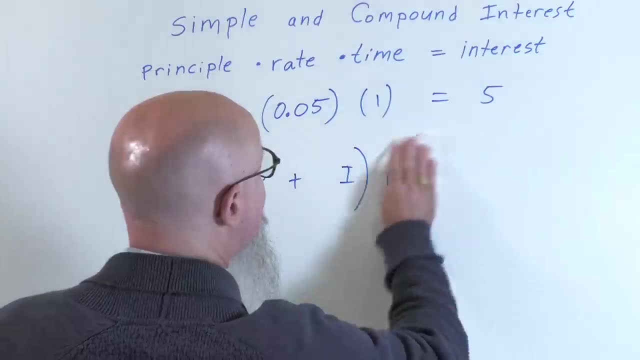 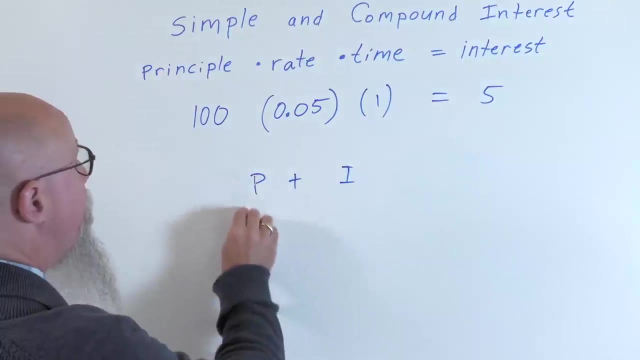 here. So if I have this, the original principal plus the interest, and I probably don't even need the parentheses here. So the principal plus, but remember the interest was principal, times, rate, times, time. So we're doing a little bit of substitution there. So the compounding part principal. 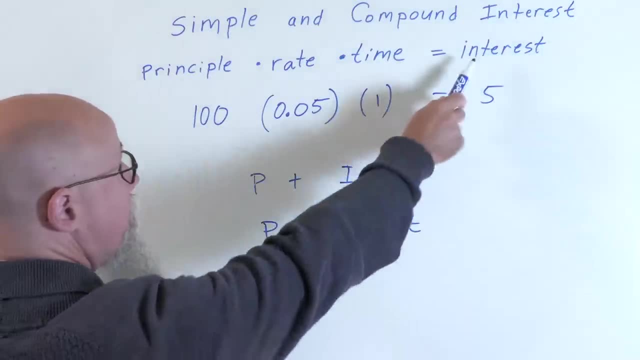 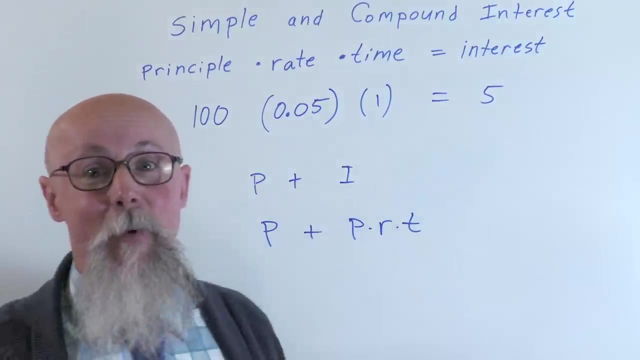 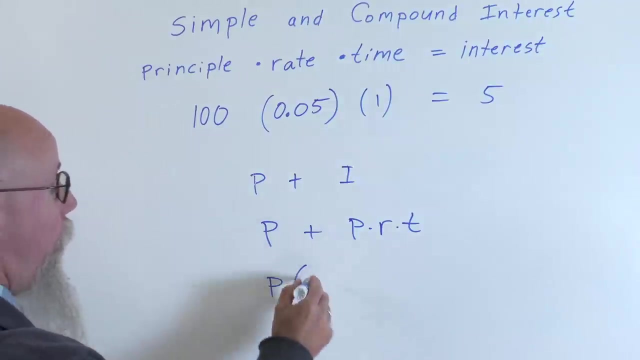 plus the interest. but the interest, remember that was this formula, So I'll just put that in here. And notice: if I factor out p- so you see the things we were doing before with common factors, factors that comes around again- then I factor out p times 1 plus rt, but supposing t is: 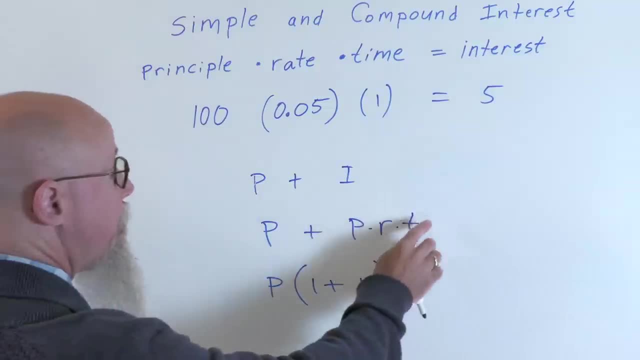 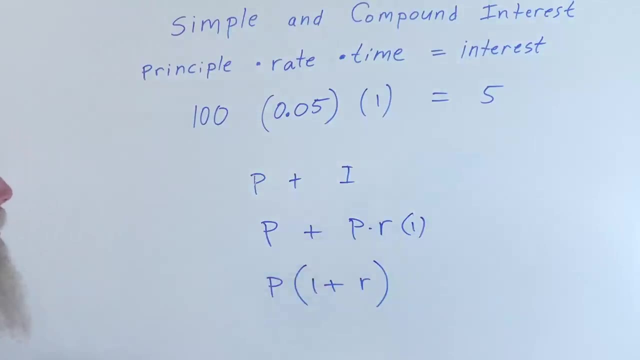 1. If t is 1,, then that would be r times 1, which you know times 1, I really don't have to write that, and then I won't write it in this step. So we see a nice algebraic way. 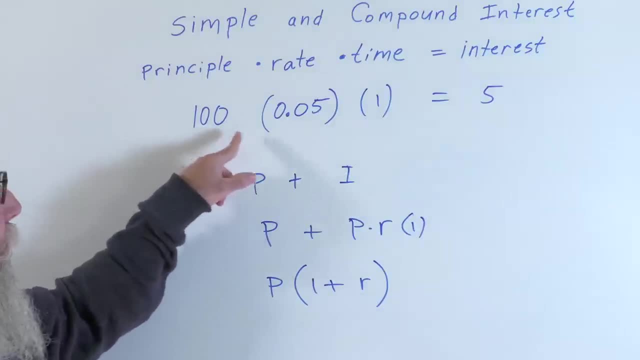 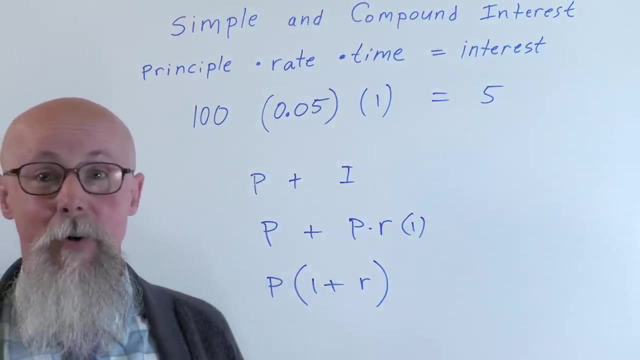 to write this, where I have the original calculating the interest and then also adding it. Now we're not going to stop there. What makes this really useful? Because that is now my principal: calculating the interest for that one year, and then now that's my new amount. 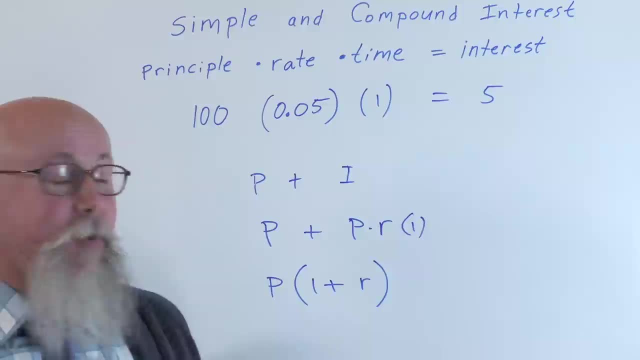 What happens when I have to calculate it for the next year? Well, what did I do to the original principal? I did principal as what I started out with and then I did times 1 plus the rate. So if I had to do it again for the next year, it would. 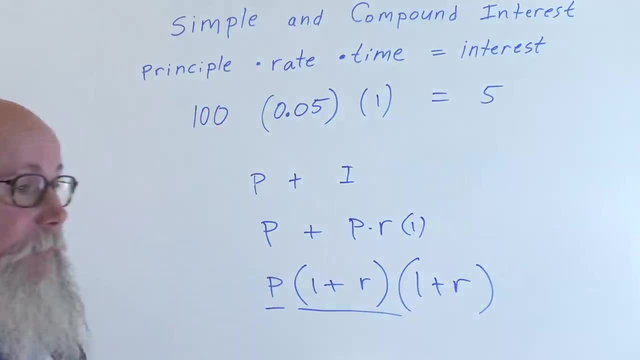 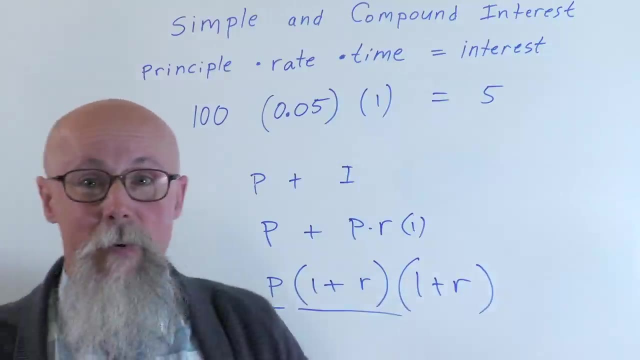 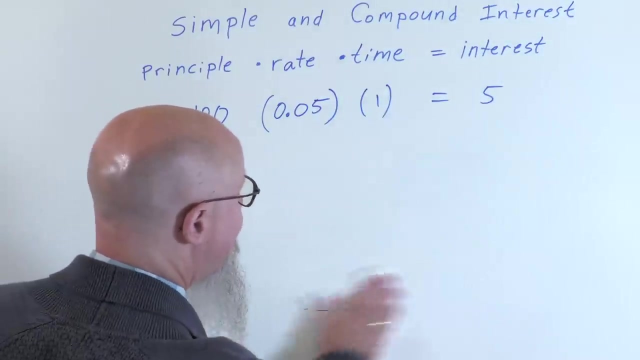 be times 1 plus the rate again, because that's what I did to get the principal plus the interest, and then again times 1 plus the rate. And when we think about this in another way, it really makes sense, because we're saying that that principal times 1 plus the rate is that 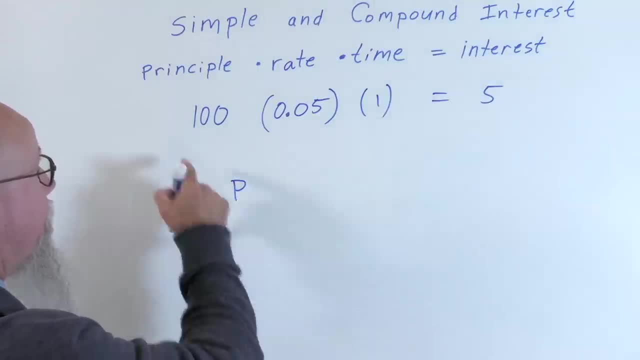 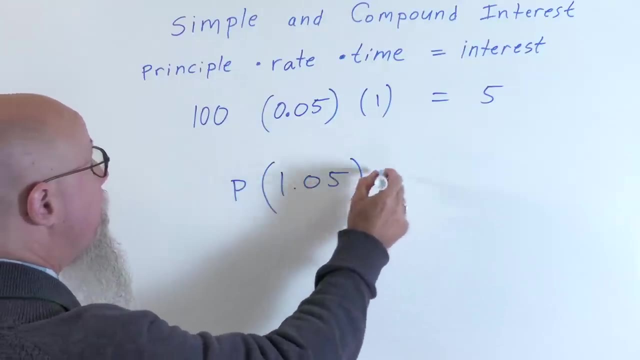 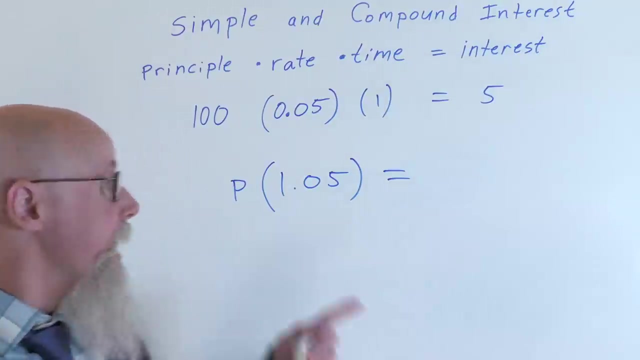 I'm saying, you know this original principal $100 or whatever it is, if that rate is 5%, you know, then that's 1.05.. So you know what do I have? I have 100% of it plus the extra 5%, And then doing that, you know that. 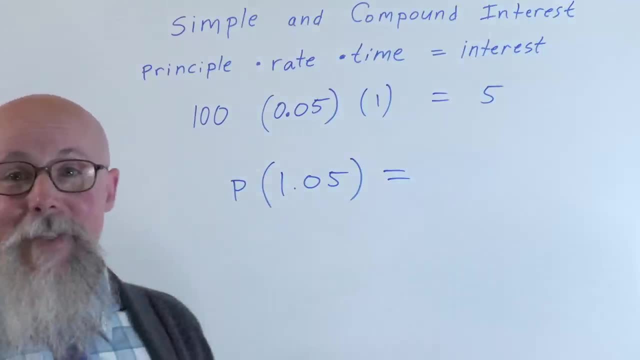 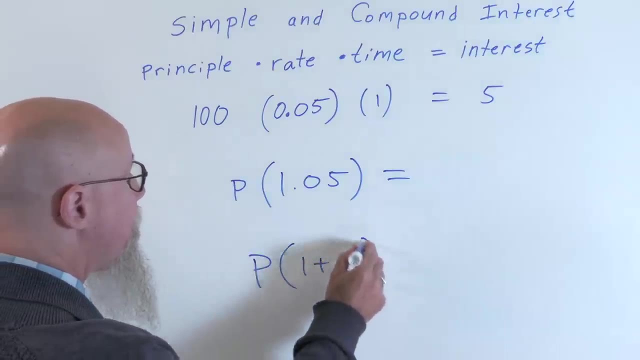 105% every time. we can even simplify this: that principal times 1 plus the rate, because if that's what I'm doing every time, how can I simplify that With an exponent? And that's where time comes back in. I have 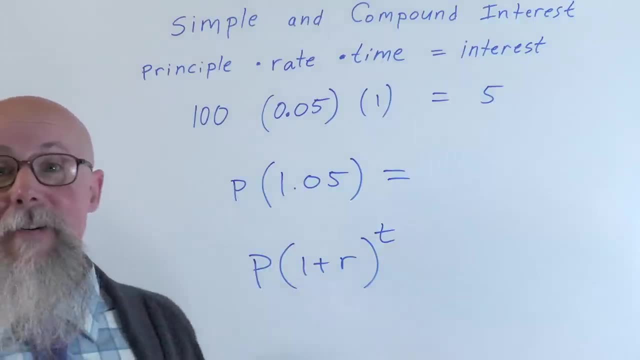 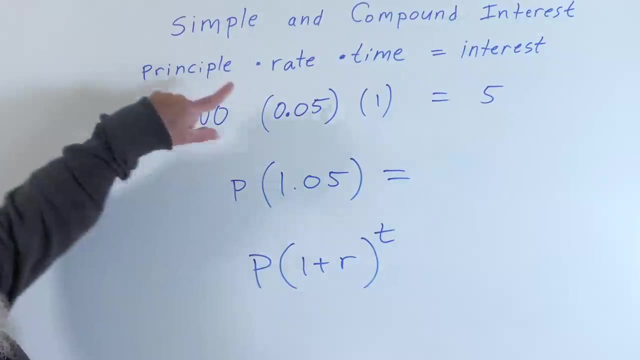 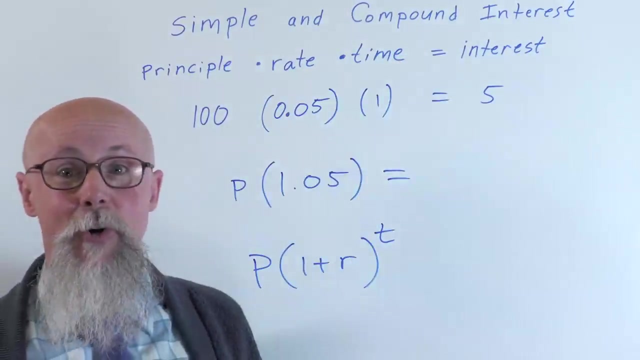 that exponent of time, because every year then I'm doing that: times 1 plus the rate, times 1 plus the rate. And so now we get from simple, which is nice, principal times, rate, times, time, to get just the interest and again, good for a short term, But you see, on long 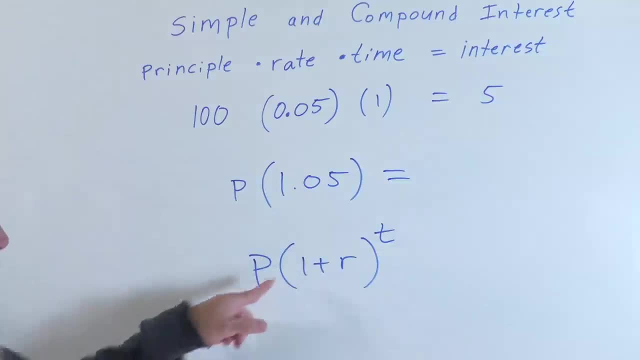 term. this is the formula that we want, that compound interest, Because that accounts for every time. it goes a little bit that I earn some interest, but then that becomes a part of the new principle and then that's earning some sort of interest. And if this was my money in the bank, that's great, that's good. 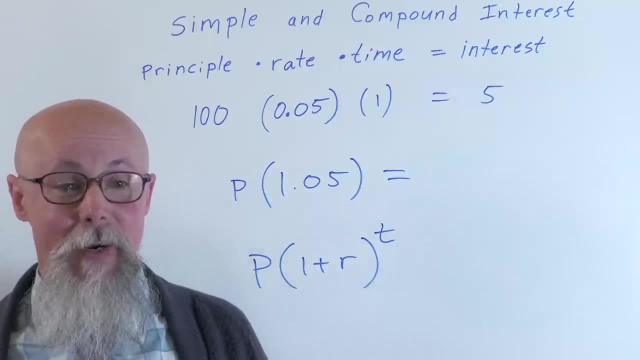 news for me. But then if this is money that I'm borrowing, then the bank is going to be wanting to do this sort of formula to make sure that they get all the money that they deserve, You know, and then I have to make sure that I pay that extra interest, So that's. 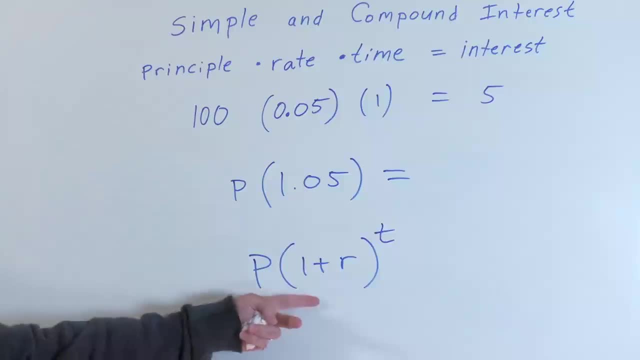 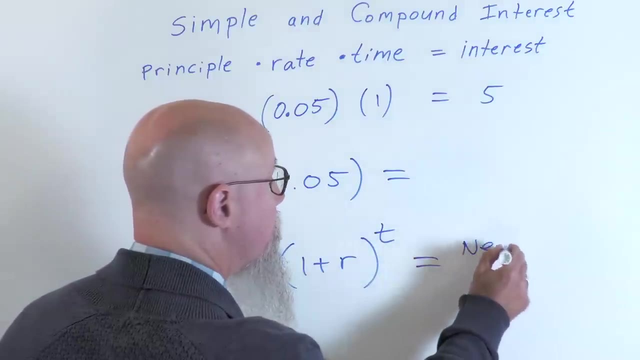 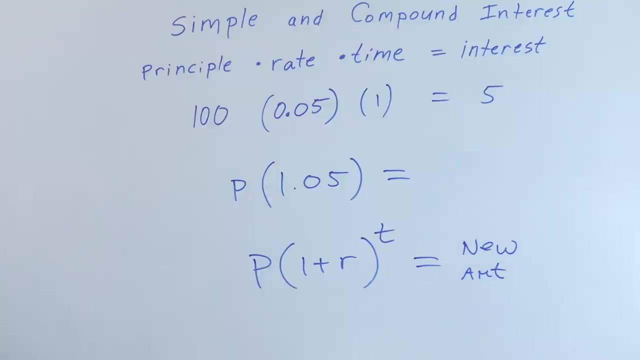 where we get the principal, simple and compound interest, and then we get to this: So then that's the formula, and then that gives you your new amount. So there we go, a new amount, And then, when we get to the code we're going to talk about that. 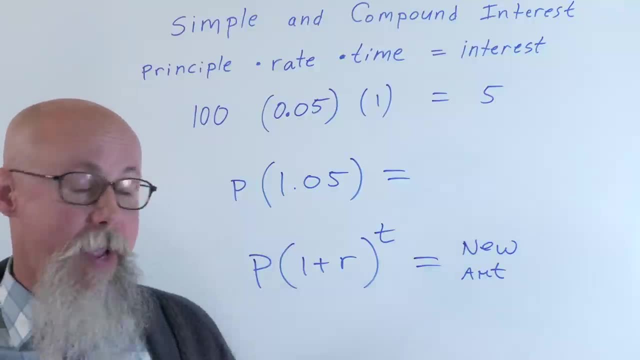 new amount. We're going to call it annuity. We're going to call it A, maybe as a variable, A for amount, but then it'll be annuity, which is a fancier word for the amount that we end up with. 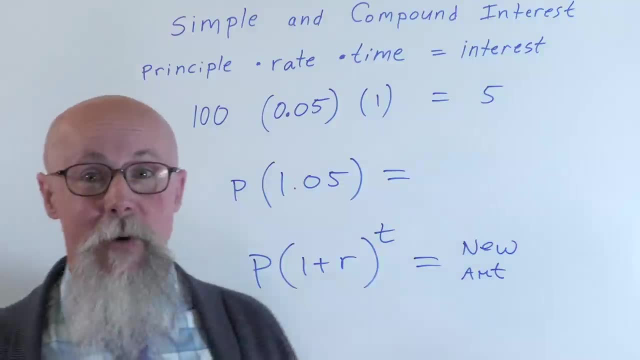 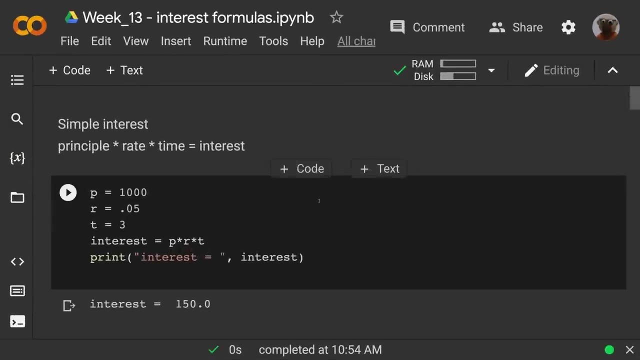 So there we go, the connection with simple and compound interest, and we'll take this a little bit further when we get into the code. So let's take a look at that, Let's take a look at the code. So we're looking at simple interest, as the well as the name says. simple because 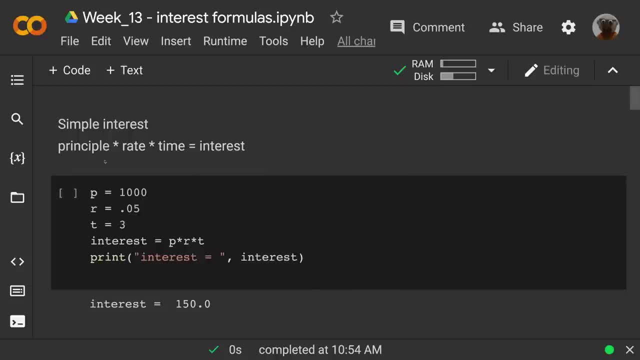 it's good for short term and for some things it might be good for an estimate, but we just get principal times rate times time equals the amount of interest, And there we go again. short term because we're going to do some other things to it. 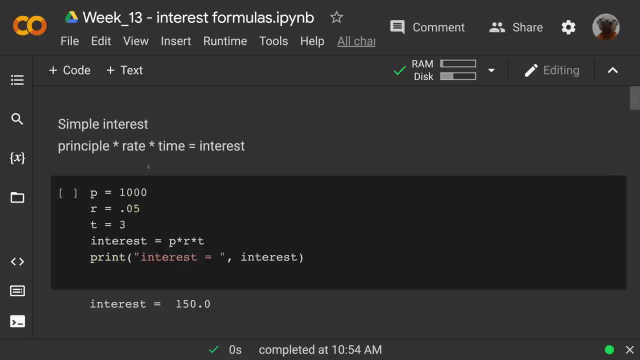 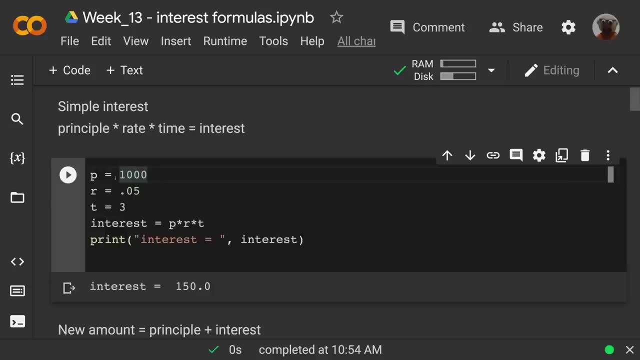 when we get to longer term and that's what we'll get to here. So the principal, if we just put some example numbers here: $1,000, let's say I borrowed money from the bank. $1,000, the rate 5%. 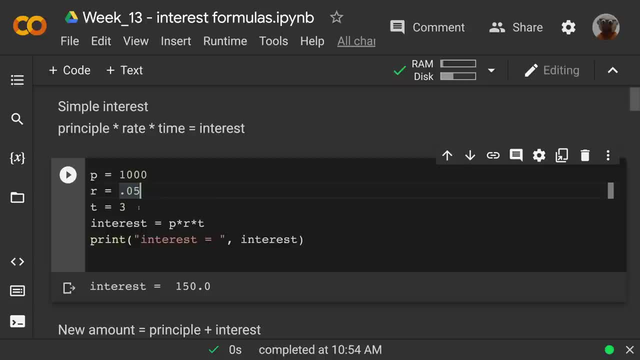 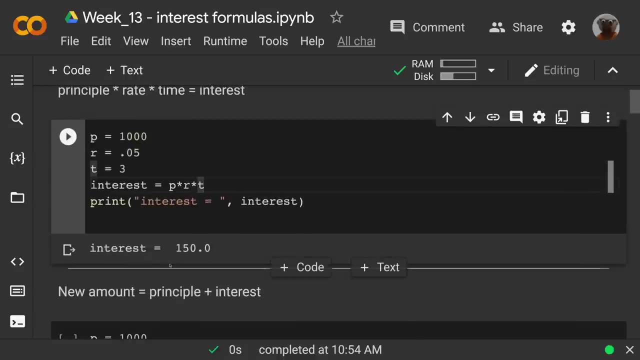 so it's always the percent, the annual rate, converted to a decimal, and then time is always in years. So if I borrowed $1,000 from the bank, they said, okay, it's 5% interest for three years, I'll pay it back. Here's the formula: interest equals PRT, and when we run it, there we go. 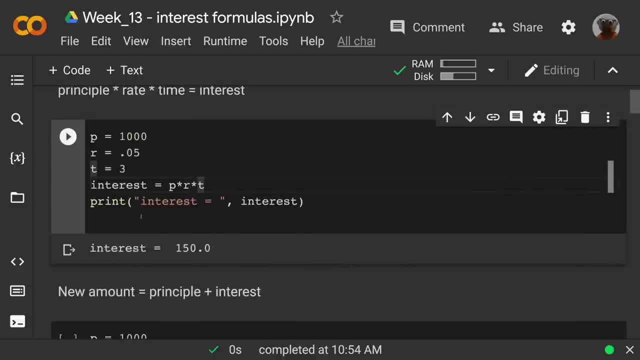 we get $150 in interest, So I'd pay back that $1,000 plus the extra interest. but right away then that tells me the cost of borrowing that I need it now and I don't have it, so that's going. 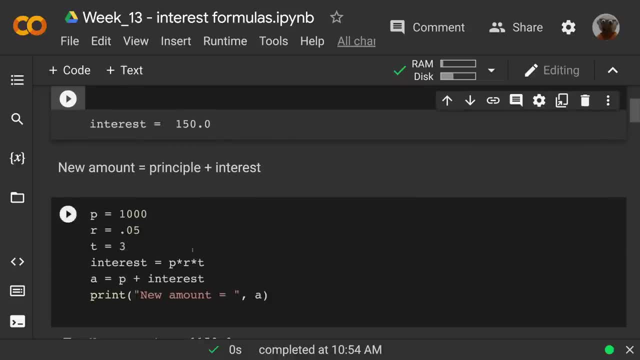 to cost me $150.. So then I want to find out the total amount. Well then, the new amount is just that principal plus the interest, and there we go. I'm going to calculate the interest just like we did before, and then 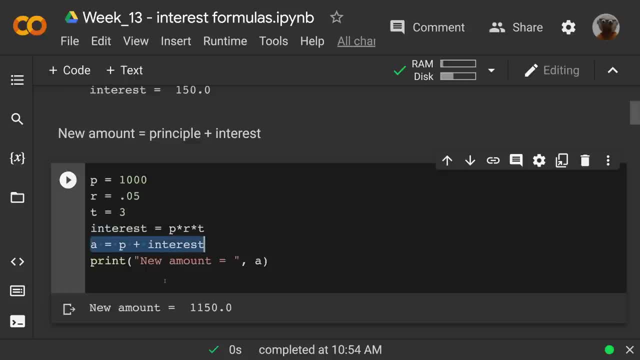 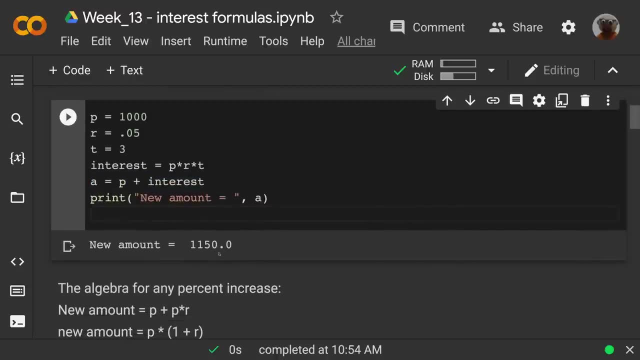 this new amount is principal plus the interest. So there we go and we add that that $150 plus the $1,000 makes it $1,150.. So now I have that new amount. Okay, so most of the time we're. 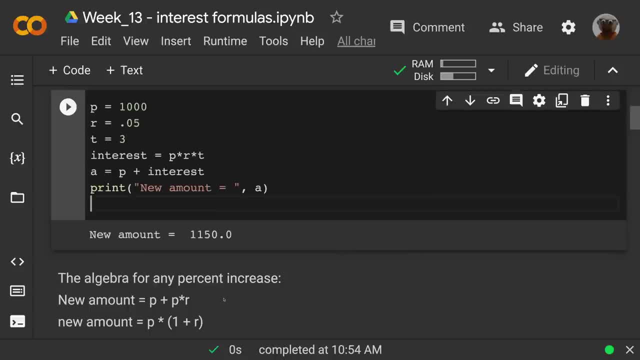 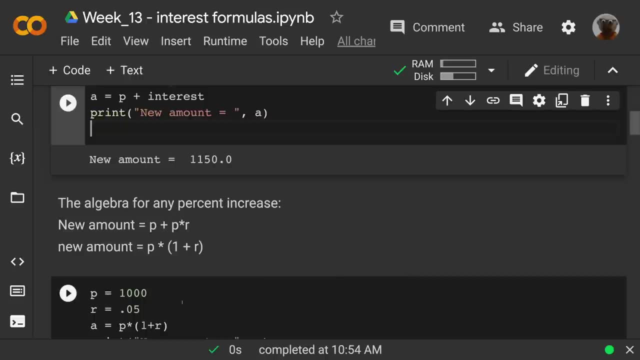 going to be calculating the interest, and then we're going to calculate the interest and then adding it to the new amount. It's very rare that I'm paying just the interest or somehow just the amount and not worrying about interest. So here's what we were just talking about: That new amount. 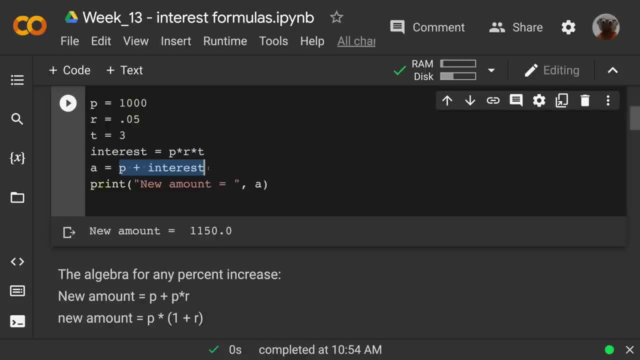 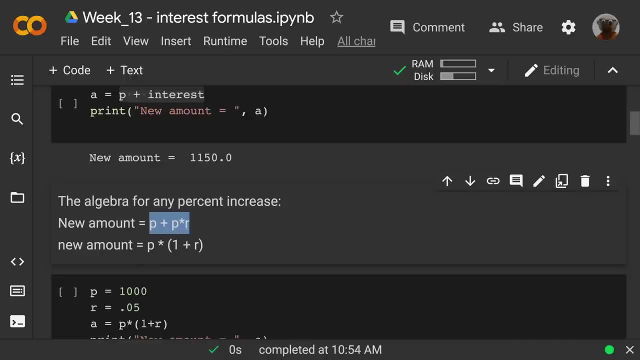 is that new amount is principal plus the interest and if it's for one year, that's principal plus. for one year that would be P times R times T, which would be one. so that won't change it. So that would be the new amount, principal plus the interest. 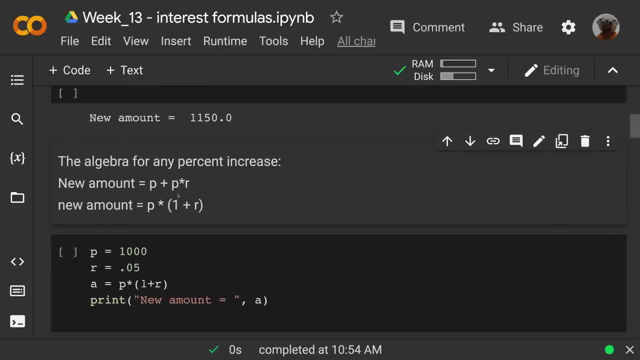 So some algebra, that common factor P. if I divide that out I get P times 1 plus R, And if I do the distributive property I get back to this. So P times 1 is P and P times R is PR. 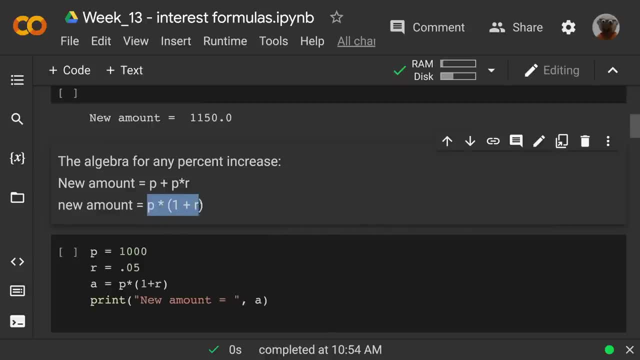 Now this is going to be very useful that we factored out this P, because now I have that new amount, just that original P plus r, and the rate is always going to be some decimal. that it's going to be pretty easy to add. 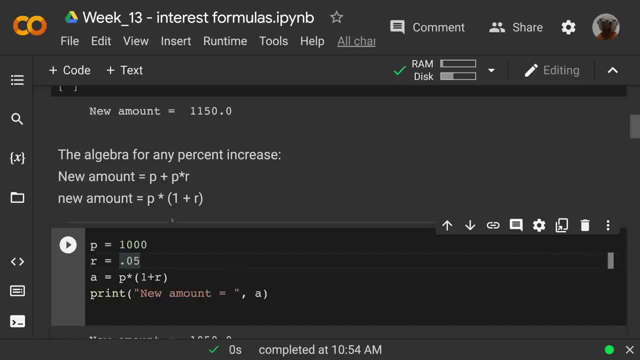 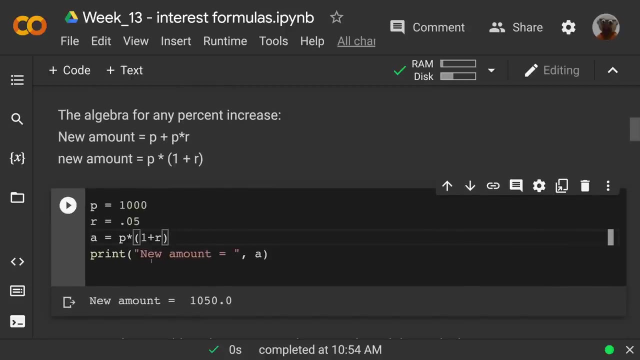 that to one. one plus 0.05 is 1.05. you can do that in your head. it doesn't even feel like a step, and then this is what you're going to enter in the calculator. so there we go. like it, one step that you automatically would do in your head, and you're most likely going to have the calculator. 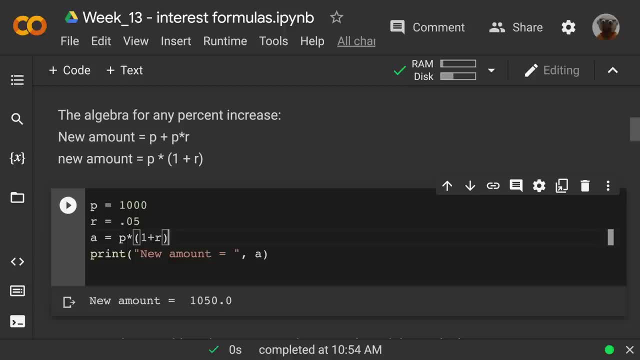 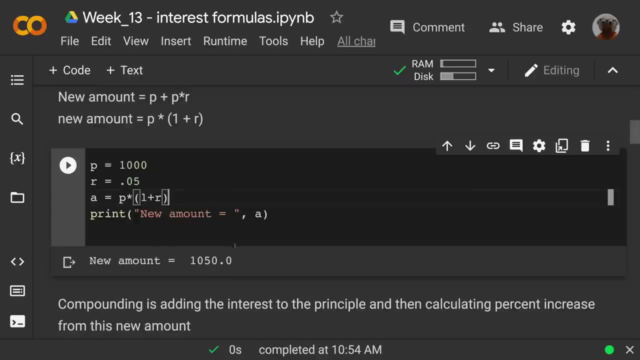 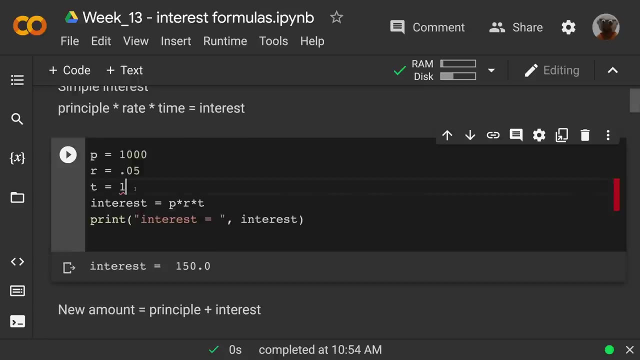 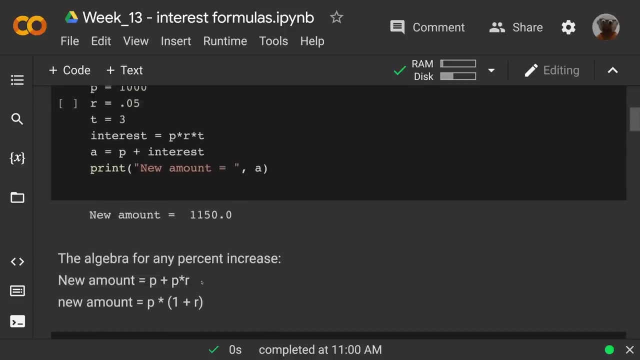 for these. so that was what you would enter in the calculator: p times one plus r. now again, this is for one year and 50. so if we go back to that original, supposing the time was one year, just to show you that this works. one year that'd be 50 in interest, and for one year then. then the new. 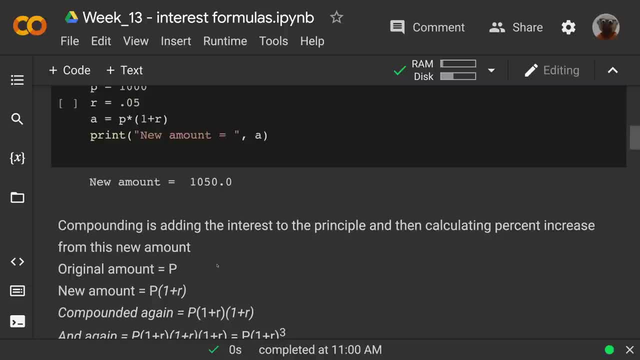 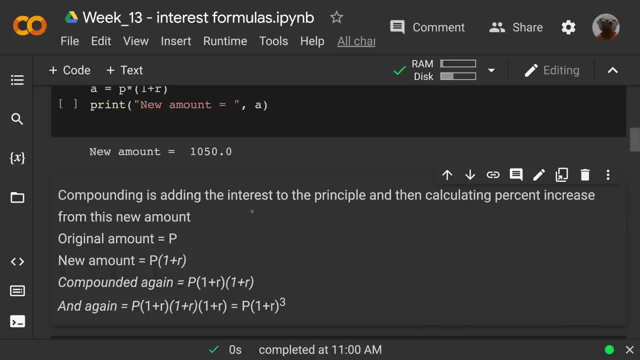 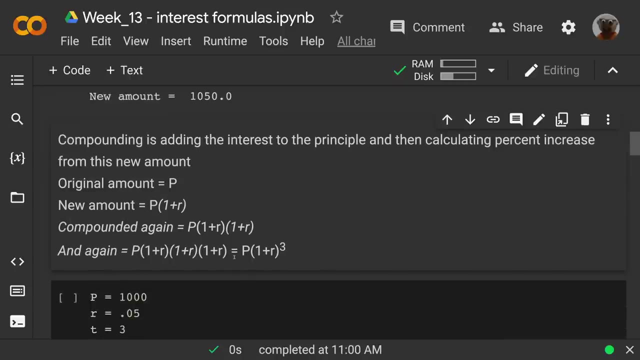 amount would be 10- 50. So that what we're doing there- adding the interest to the principle- that's compounding. and compounding is exactly that: adding the interest to the principle and then calculating the percent interest from this new amount. so let's look at how this happens over a few years. 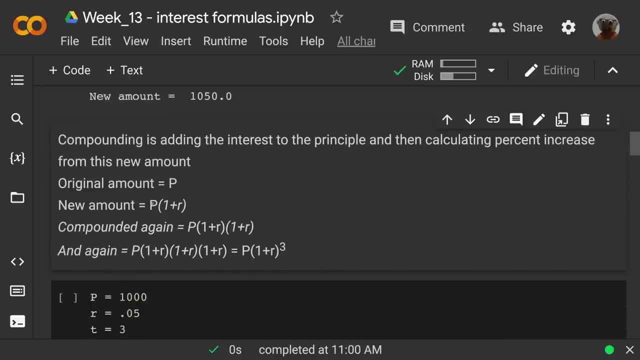 so if my original amount is p, so then the next year it's p times one plus r. but now that's my new amount, so so again the next year. so p is the times zero. After one year I multiply times one plus r, And after another year I multiply times. 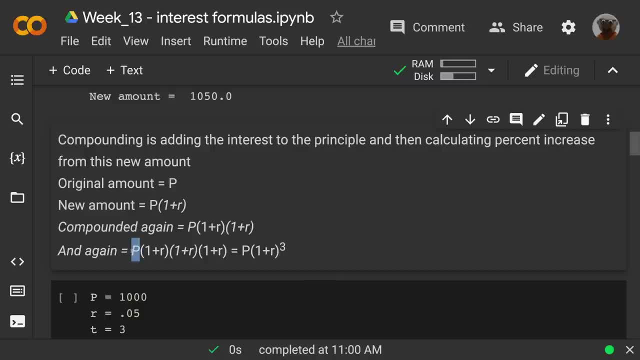 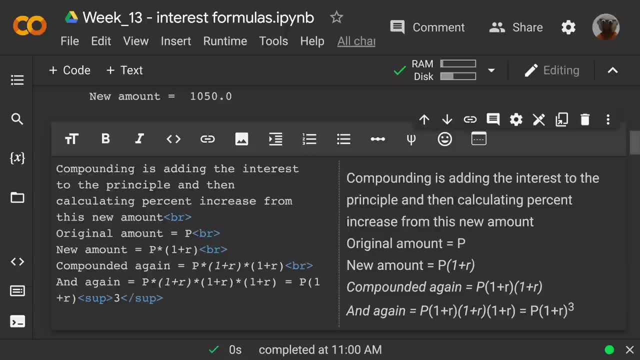 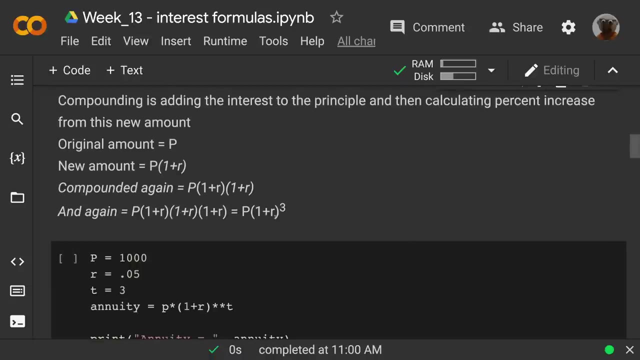 one plus r again, And we'll just do this one more And again: p after one year, after two years, after three years. So then that's just the same as making this an exponent p times one plus r to the third power, because I'm multiplying this factor one plus r three times, And now we have 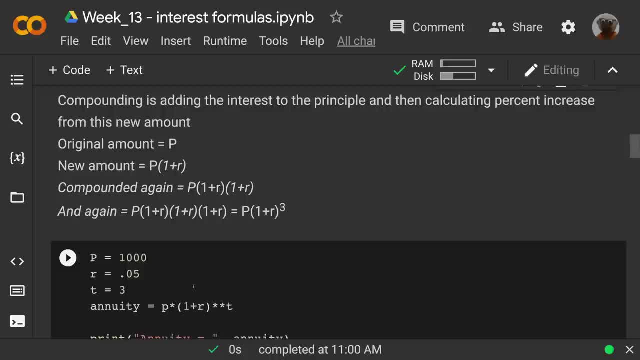 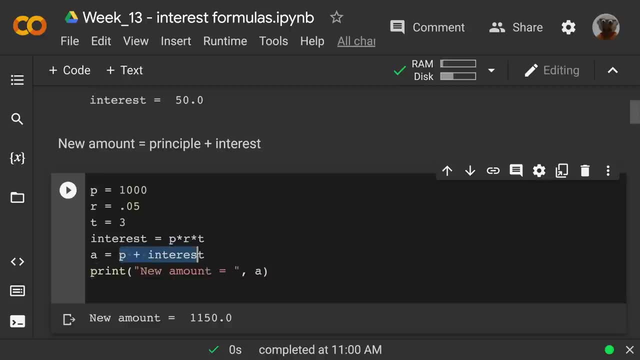 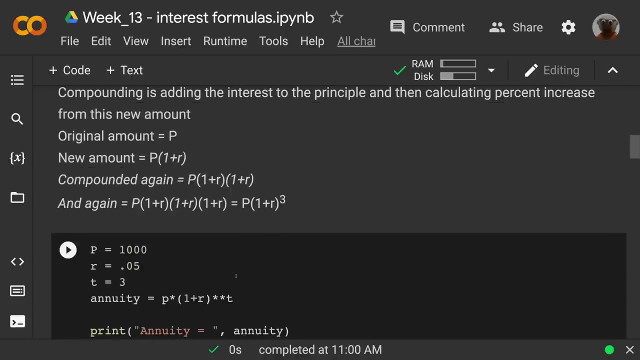 compound interest that instead of having to go back and every time calculate the interest, simple interest, add it and then do it again. you know, in some loop I have one formula that does the compounding And all I need to do is add the exponent: for how many years? 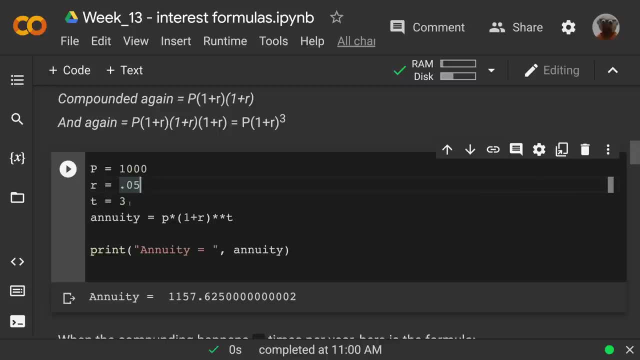 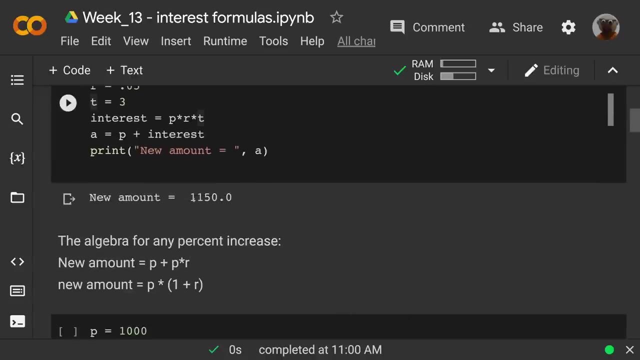 So now the annuity from the original: p times one plus r exponent t, So that's 1157.. Now, it's not an error that this is different, And remember the original was 1150.. When I did this by hand, I just, you know, calculated the interest based on simple. 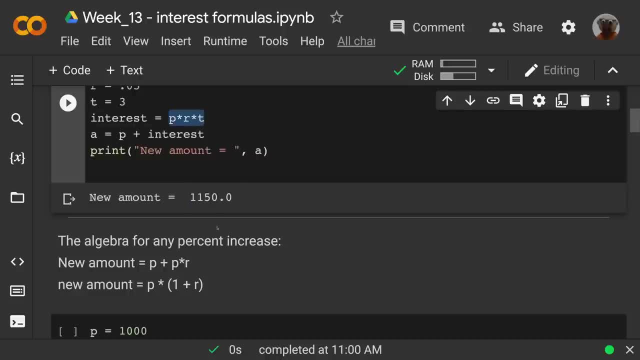 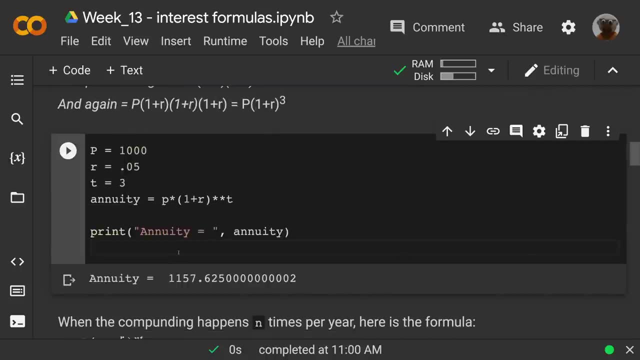 interest and then added it, But that's after three years. it was 1150.. And, like I said, simple interest is good for short term, But the longer it goes, the less accurate it is. So when I have this come, when I'm compounding it every year, notice that's every. 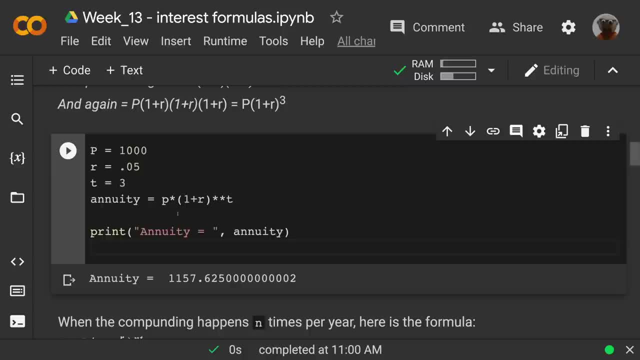 year that I'm adding the interest, And then the next year. So remember, after after one year it was 1050.. So then for this, for year two, I'm getting that 5% interest on, not on 1000, but on. 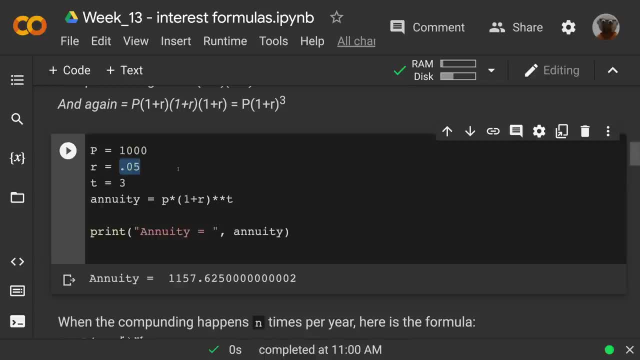 the next year I get that 5% interest on that new amount. So that's the compounding. It's like a snowball that rolls down the hill and accumulates more snow and gets bigger and bigger as it goes down. That's what we're doing every time we're compounding, because I'm still taking that rate. 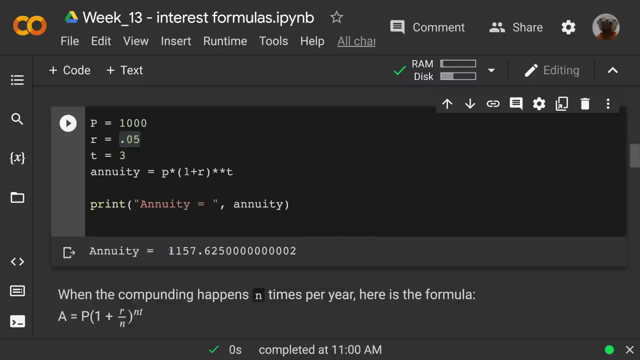 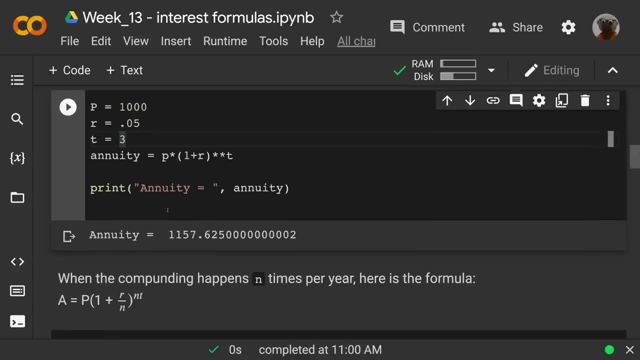 5% of a larger and larger amount. So compounded I get 1157.. Just that same amount over three years. I earned an extra $7 just because the formula was better. So time is always in years and that's compounding every year. 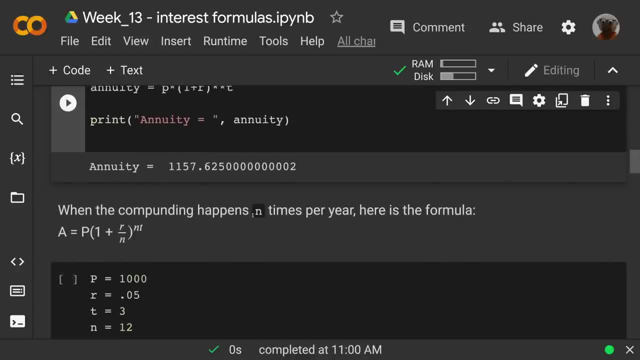 But we also have a formula, supposing compounding happens n times per year. So that gives us this more complicated formula. But that's okay. We see how it connects P times one plus instead of R. we're doing R over n because this is happening n times per year. 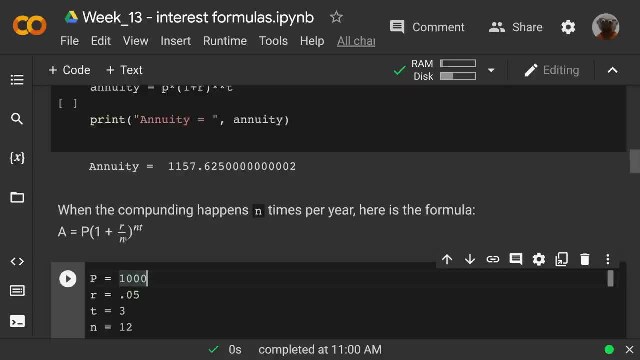 So that rate isn't always an annual rate, So I have to divide it by how many times I'm recalculating it. But since then every year was the exponent? the exponent becomes NT. how many times a year times the number of years. So then I'm compounding however many times. As an example here I put: 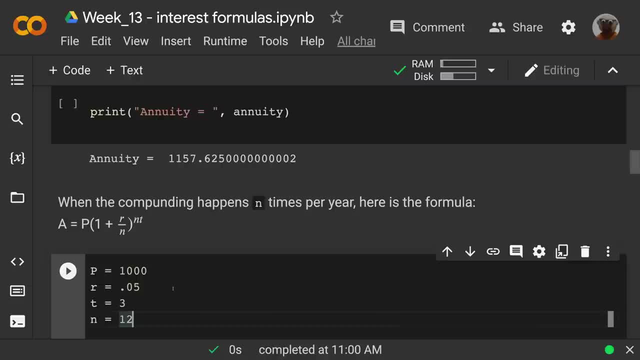 it as 12. Because that's pretty common. Monthly, we know, recalculate, compounding 12 times a year. So then one plus R over n- what's in these parentheses- gets smaller, but then the exponents larger, and it still ends up working out: if this is money, Now, if this is money you're. 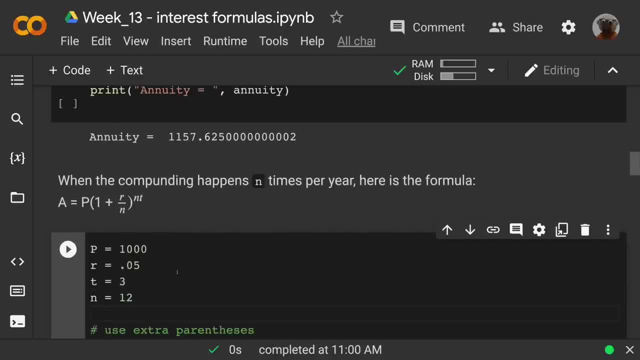 paying back, it ends up paying. you end up paying more. But if this is money you're putting in the bank earning interest, then it works out in your benefit. So that thousand dollars, five percent, for three years, but now this time compounded 12 times per year. 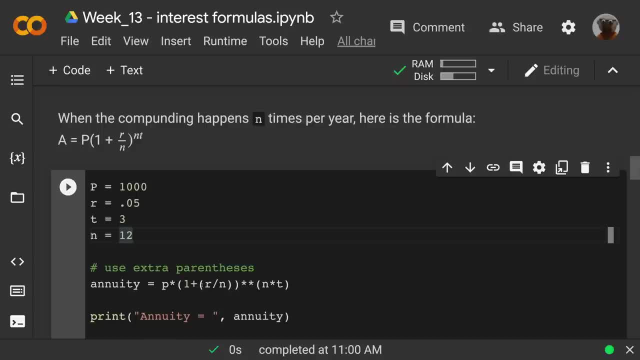 I use the extra parentheses for any fraction. so there you go. instead of just r, here it was 1 plus r over n. I put that in parentheses also, and you definitely need the parentheses here to make sure that stays, because that is the whole exponent nt. and remember the python syntax. 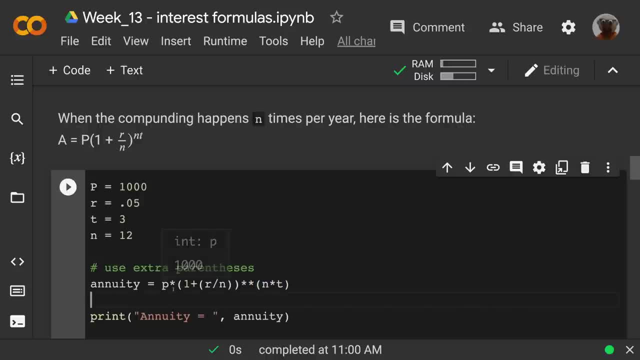 you know, in math we might skip the multiplying symbol because we're just, they're next to each other, but in python have to put that asterisk there. so there's the annuity. um, the other thing. we're going to talk about this, instead of just amount, that's annuity and principle is the word. 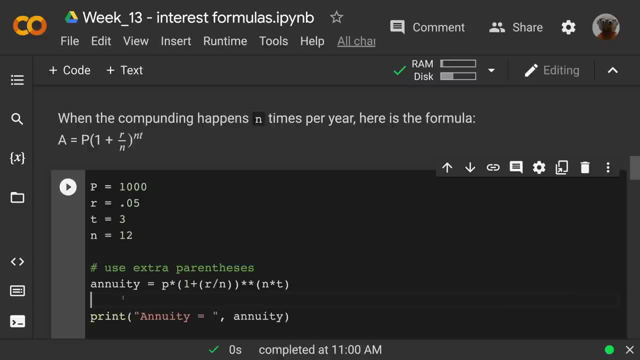 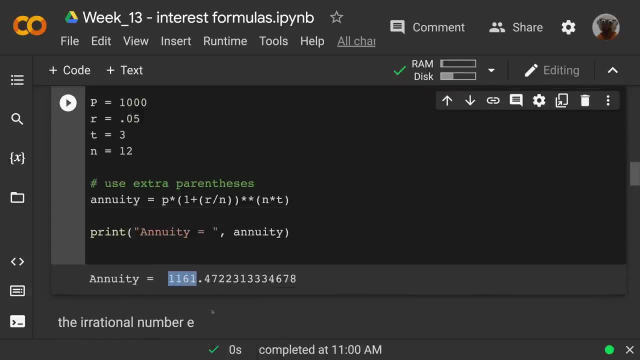 for the amount we start out with and annuity is the word for the amount we end up with. so now the annuity compounded monthly- look at that- it's 1161. so we go back from that simple interest and we go back to that simple interest and we go back to that simple interest and we go back to 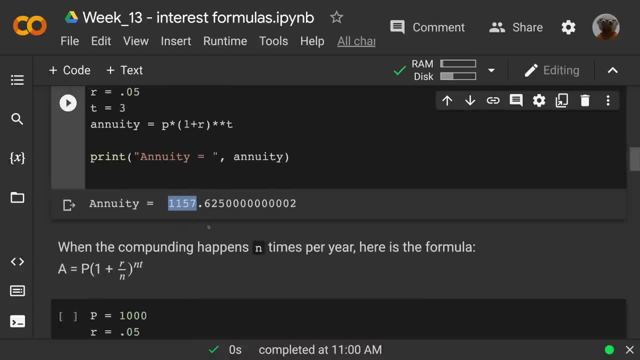 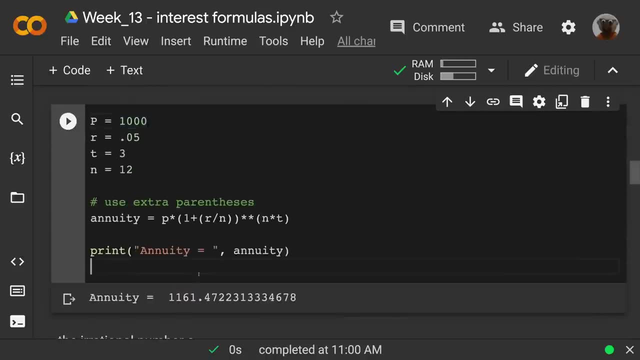 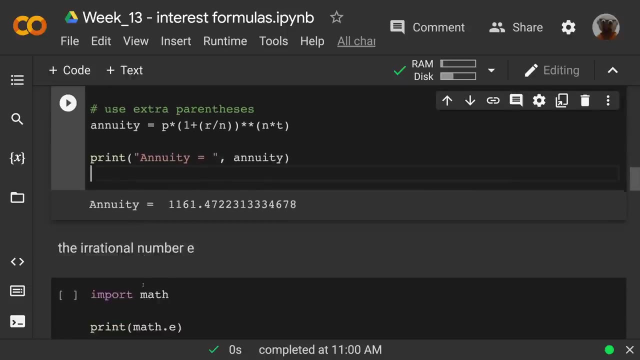 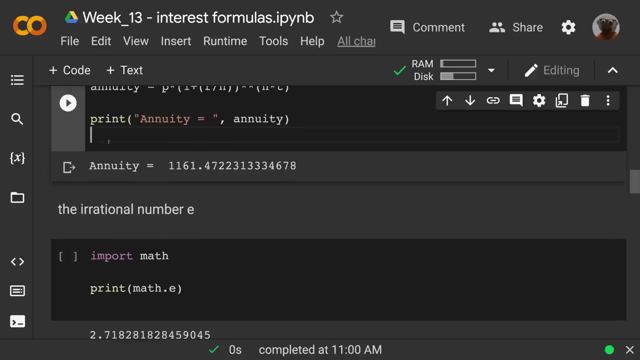 that was kind of off to compounded annual 1157, much better to 1161 because we're compounding it monthly and guess what it gets better. but first I'm going to start talking about this irrational number e. now in the middle of all these very practical money in the bank things that we can. 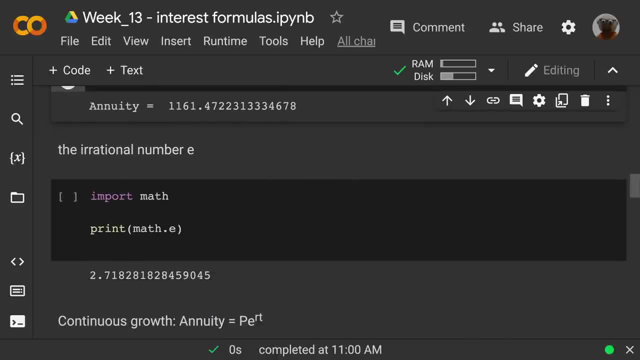 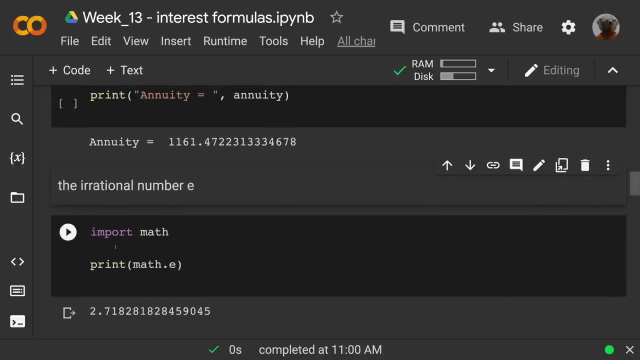 understand. why am I going to start talking about this irrational number e now in the middle of all these very practical money in the bank things that we can understand. why am I going to start talking about? This is going to come up in the next formula, all right, so 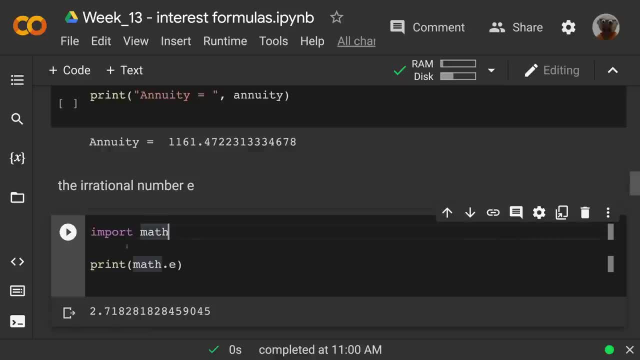 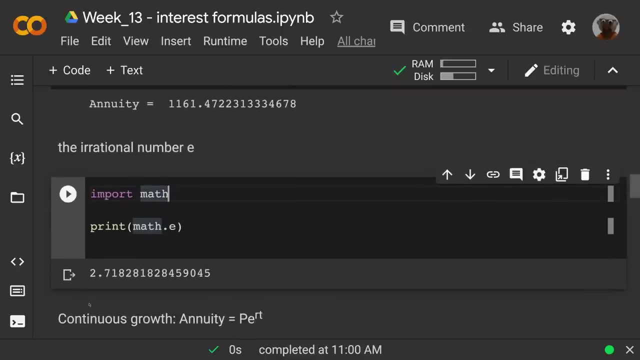 Just a quick note about eat. we're going to import math because he's a weird number and so when I print math e, this is the number For you and as a good estimate you can just called two points 7, but in your calculation you actually want to use this whole number. 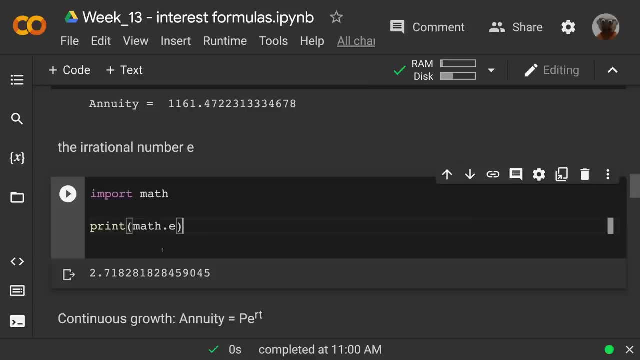 that's why I wantedition want to import mathe. I don't want to just, you know, say 2.7 and call it good. Another interesting thing about this: it's 2.7, and then we see it's 1828, and then the 1828 repeats again. I don't. 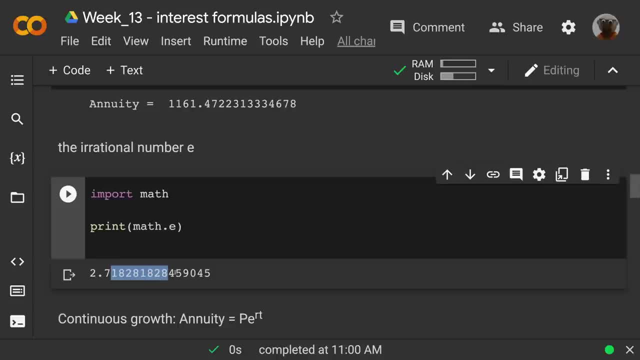 know it's kind of interesting, but it only does that a couple times and then it just all falls apart. So, mathe, use that for the irrational number e. and it's e because it's Euler's number. Um, his name began with an e, but, uh, John Napier, who invented logarithms and other things. 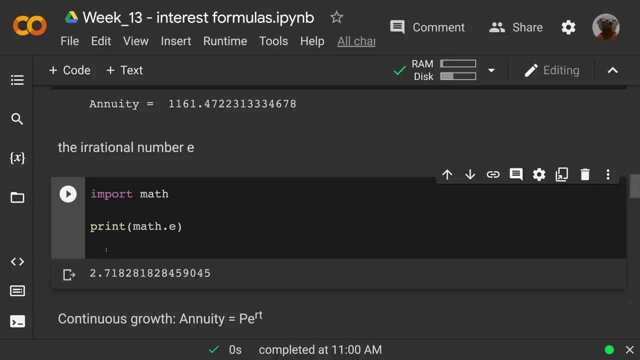 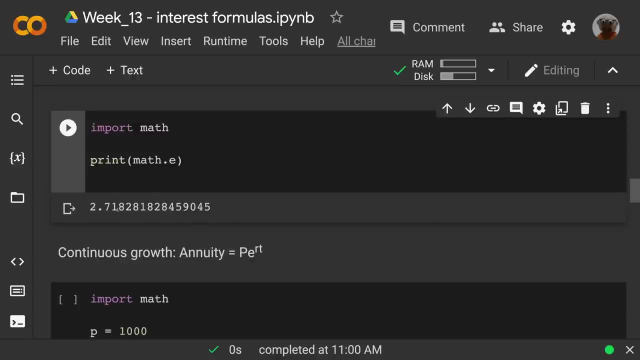 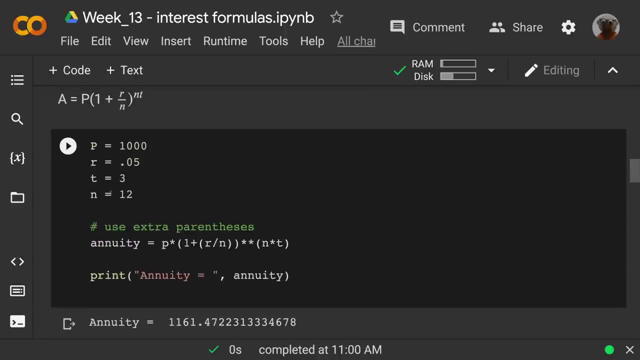 when he came up with this number, um, he named it e after uh, another mathematician that he liked, Euler, So sometimes people call it Euler's number, but anyway it's e. Now if we're talking about compounding n times per year. 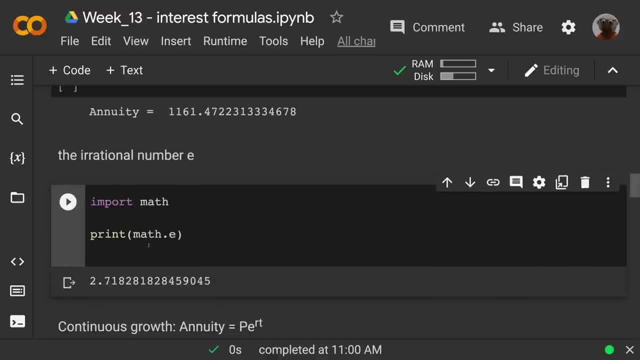 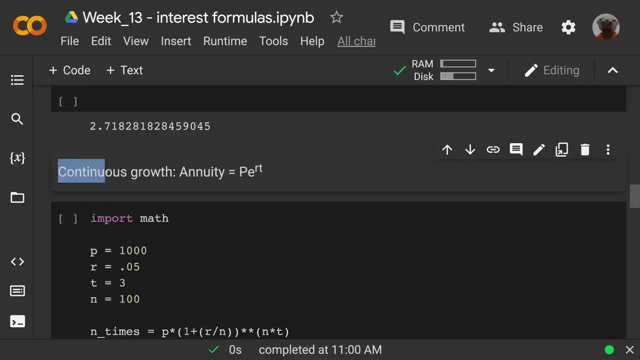 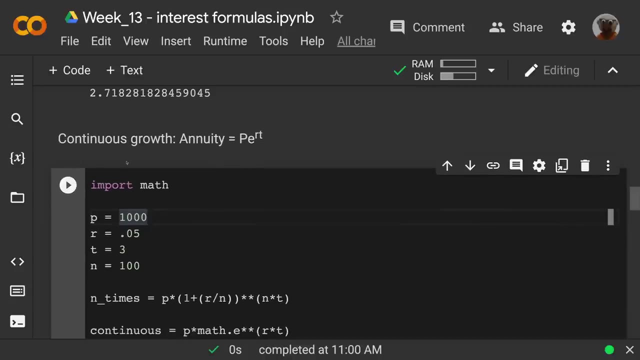 we go? we go from being irrational and talking about e to being very rational. Well, what if I just keep compounding it many times? And that's where we get to continuous growth. So in that previous formula, n could be 12.. Now, in this example, I made it 100 because we're going to do some things. 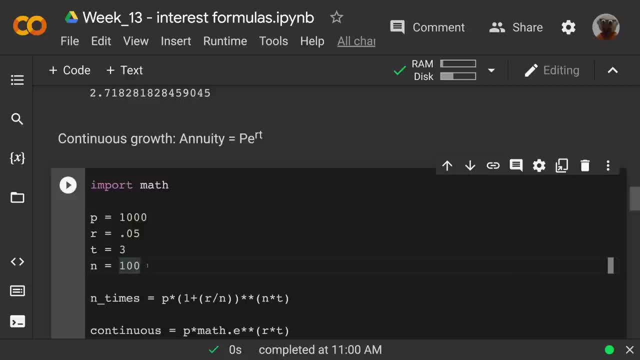 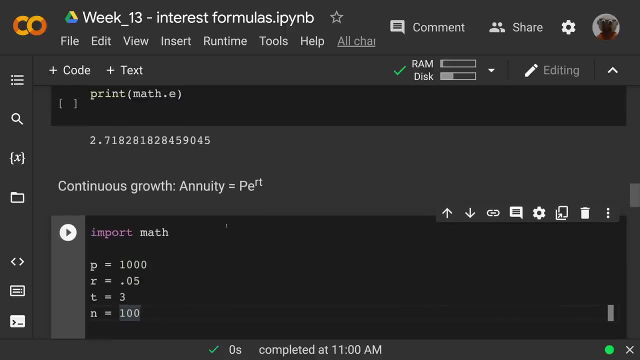 with this. Um, you know, it could be 12 every month, 52 every week. You know, I just made it a nice round number: 100.. It could be 360.. 65.. As n gets to be a bigger and bigger number, then we get the annuity becomes this formula: 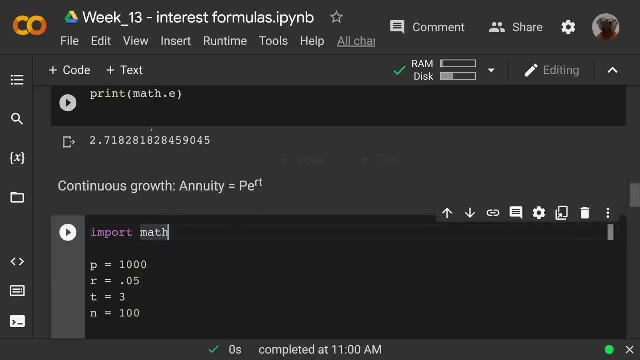 p e to the r t, And that's why we were talking about e. So I get this irrational number e, and then the exponent is r t, Because, as we get, well, I'll, I'll. I'll just demonstrate this. 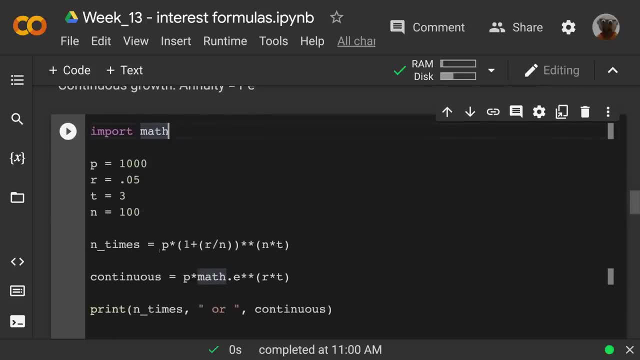 So let's say n is 100. And if we do that, um, actually let's even make it 52.. So compounding every week. And then here I'm going to compare these two formulas. So this one called the variable n times. So there's. 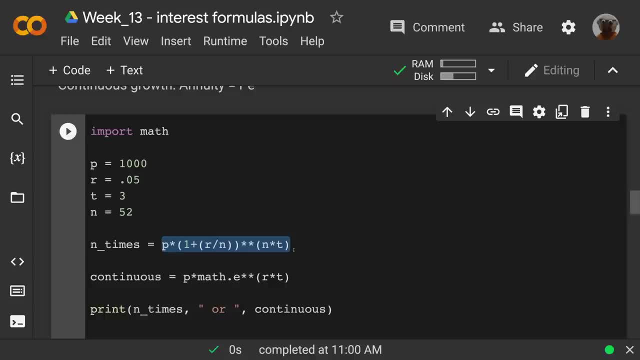 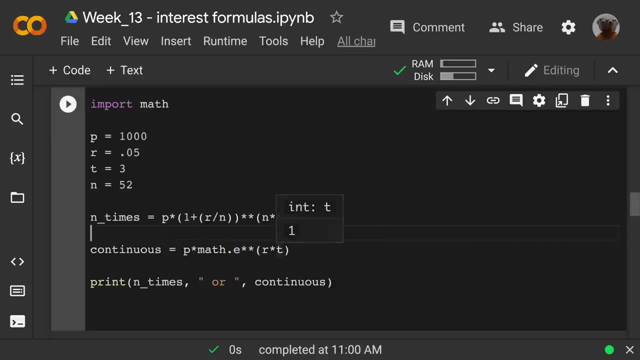 the. there's our other formula: p times one plus r over n to the n t, And then we're going to compare that with our continuous growth. p times math dot e exponent r, t. And then we're going to print it, This one: 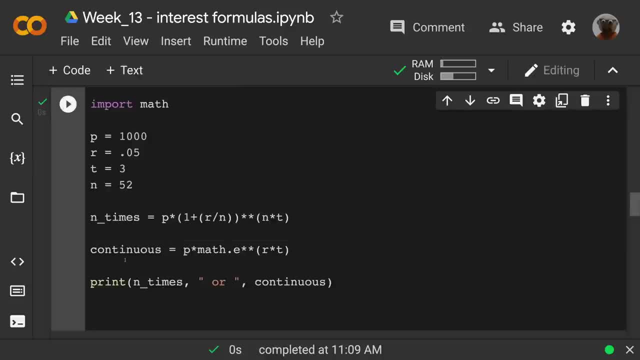 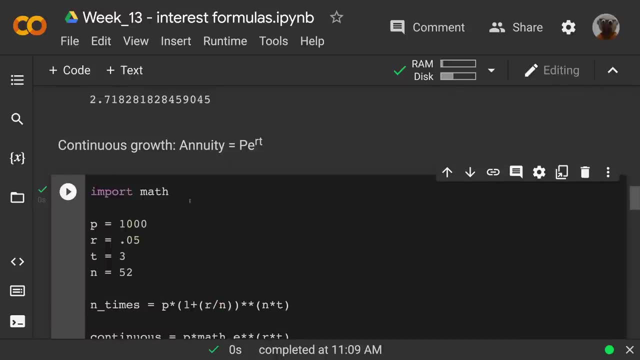 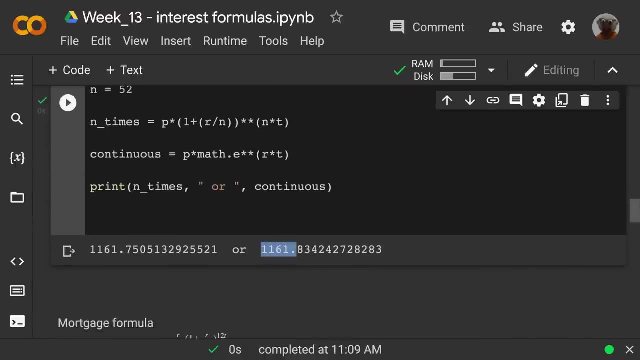 or this one. So n times we remember that from before 1161.. That should be the same number, And then the continuous growth, 1161.83.. So it's pretty close, But it's a little bit more for the. 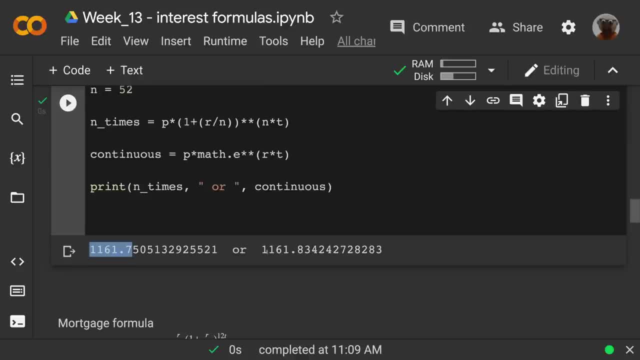 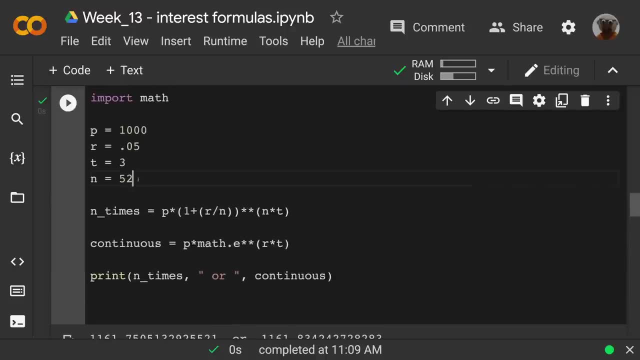 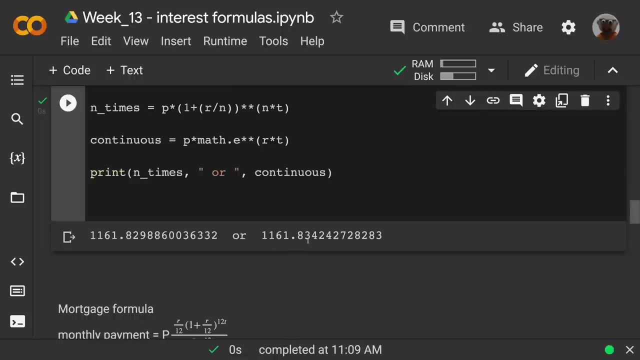 1161.75, 1161.83.. It's pretty close But the continuous growth gives us even more And if n gets to be a much larger number, like a thousand, you'll see it gets really close: 1161.829, or 1161.834.. So we see, if we took it to. 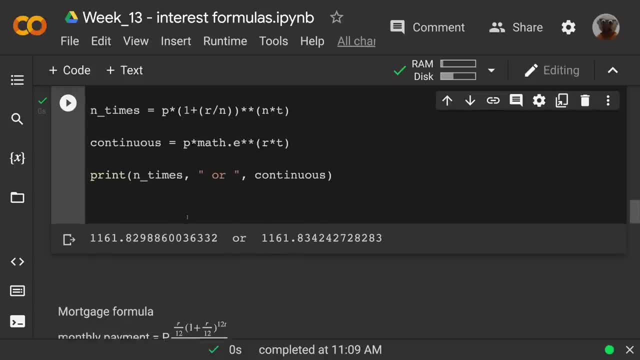 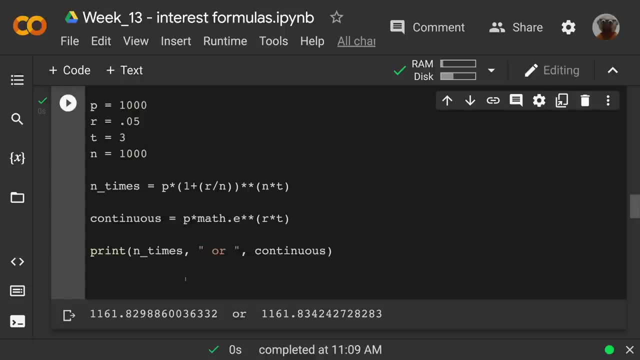 two decimal places, they actually round to be the same. Um, Yeah, Okay, That's the idea with continuous growth. You see, it's not that it's always going to be more than this, it's that as n gets larger. 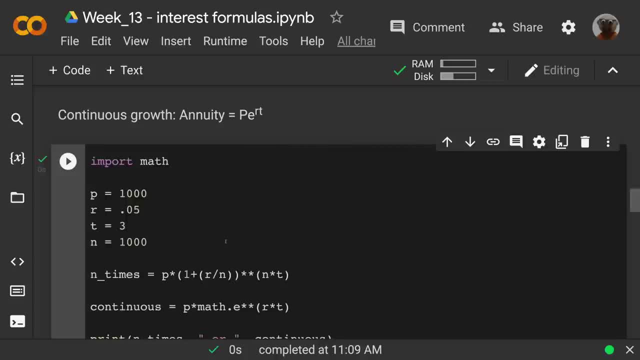 it approaches this value. So if I have anything that's compounded, a lot, or other things beyond money in the bank or things like that that I can say are continuous growth, applications, population increase or things like that, then I'm going to use this and I can call it annuity, I can call it the 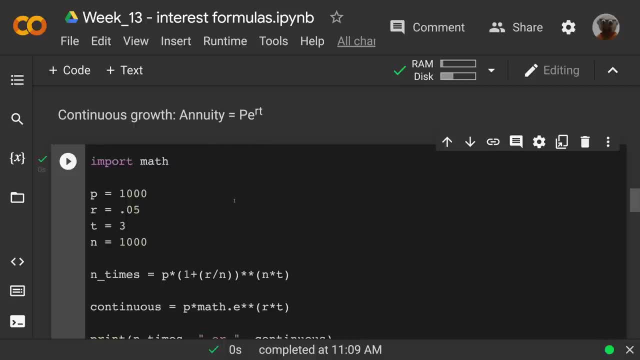 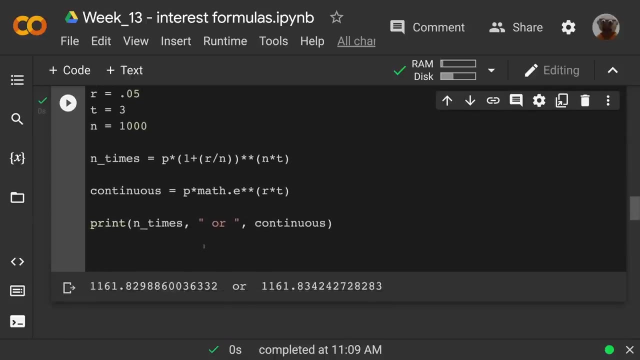 new amount. but I'm going to use this formula So it's very useful for anything. continuous growth- It comes up a lot. I mean throughout math and calculus- some version of this comes up a lot. So I have this continuous growth formula if I want to calculate this. 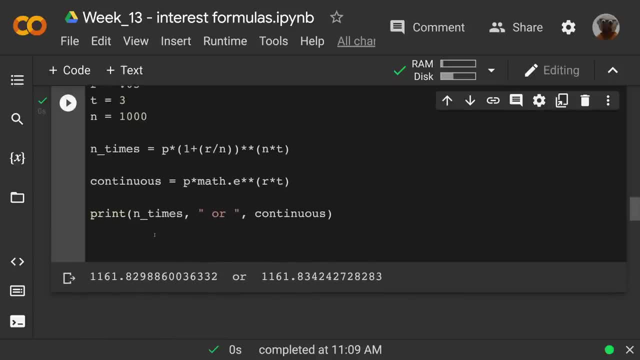 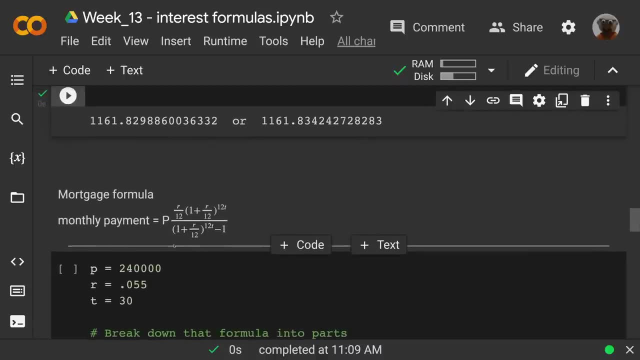 All right. So for really large amounts, the mortgage formula and the mortgage payment formula is: if I have a really large amount of money and that's usually a mortgage. as an example, I think this might be pretty close to the average mortgage these days: 240,000. 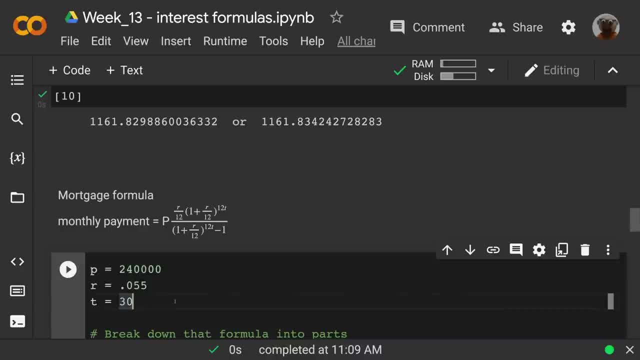 So that's a large amount of money. and then time is: 30 years, That's a long amount, That's a long time. So for such a large amount of money over such a long period of time, then it actually really makes a difference if I'm paying just a little bit. 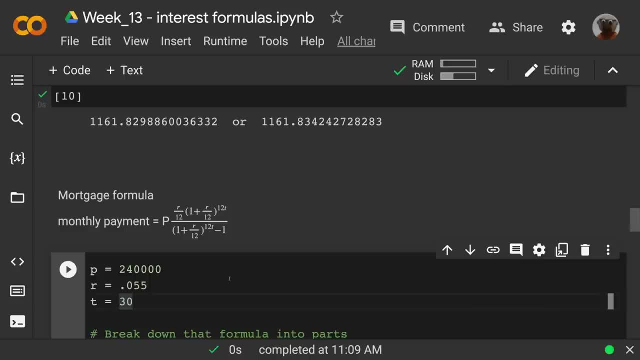 Every month. the fact that I'm paying a little bit and then that principle reduces just a little, then the next month I'm earning interest on that slightly lower principle. Well, that really makes a difference. So if we use any of the other formulas, we're going to get a little bit more interest. 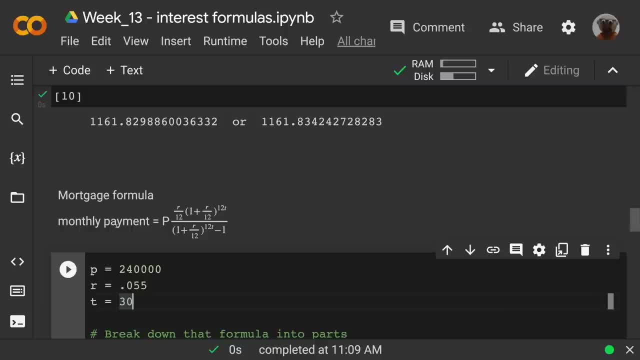 So if we use these formulas to calculate mortgage payments, it's going to be a lot more than you would expect. You'd be like, oh my gosh, how can I afford that? But when we use this more complicated formula, this accounts for the fact that we're paying. 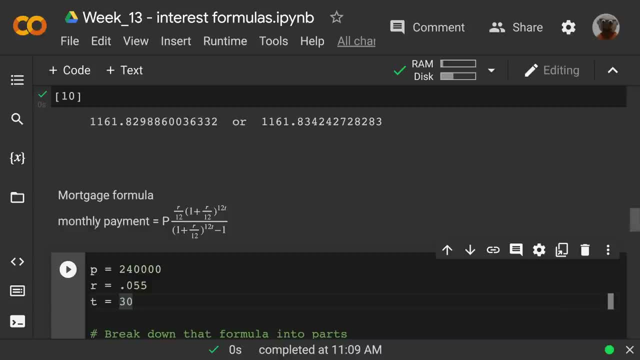 it off gradually And looking at all that, then we can take a look at for that given amount of time, what would my monthly payment be, so that it'll work out nicely, You know, Okay, So if I'm paying over 30 years times 12 months, that's 360 payments. 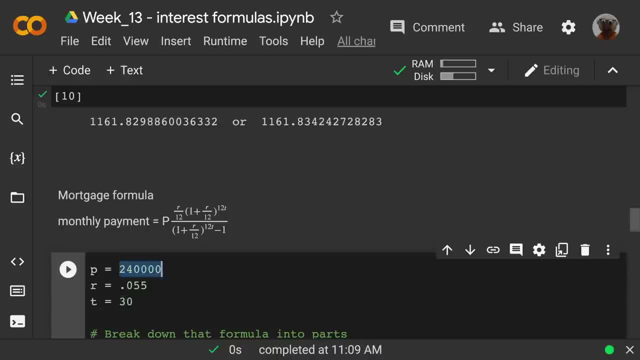 So I can calculate it: if I borrowed this amount of money after exactly 360 payments, my balance is zero and it works out. So, just given that, I can figure out the payment and then we'll look at how that plays out. So, this being a complicated formula, if we want to write code for this and most of the 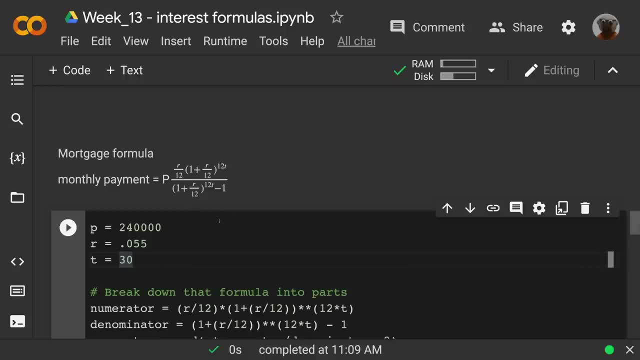 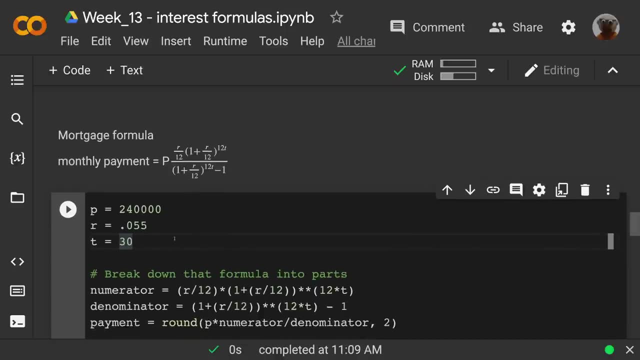 time you're going to, You don't even usually enter this into your calendar. You're going to make a formula that you can plug in the numbers here. So that's what we're going to do, And here's how I decided to break that down. 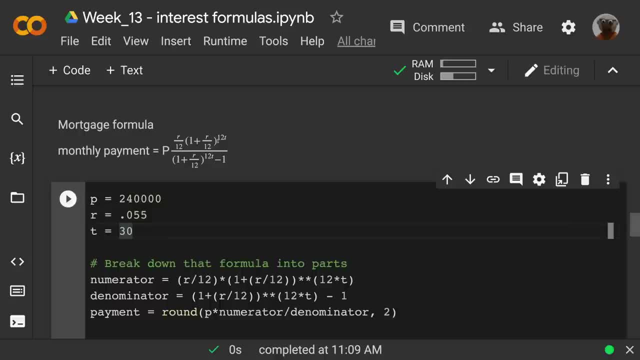 I just took the numerator that r over 12,, 1 plus r over 12,, 12t, And just that numerator. I made it a variable and we see r over 12 times 1 plus r over 12 to the 12t. 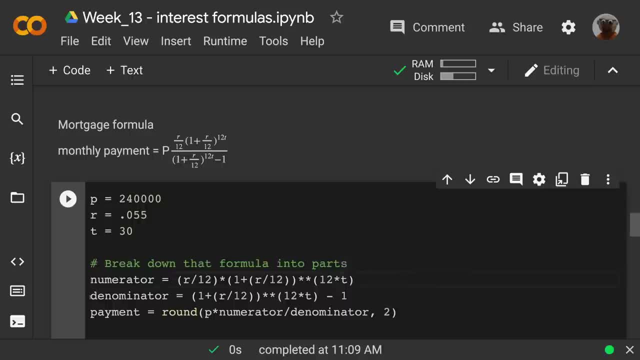 All right, And I did the same thing with the denominator. So just the denominator, and I have 1 plus r over 12, so the exponent 12t and then minus one separate from that. So I have numerator, denominator, two separate variables. 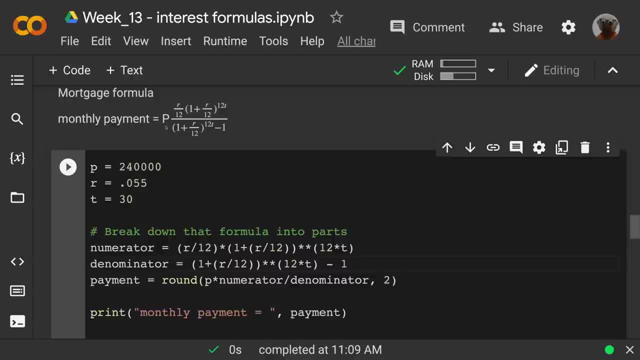 So then the payment. see, I didn't forget about that P for principal there, the capital P for principal. So I'll talk about the. so I'm going to round this because this is going to be a weird number And the first part is P times. 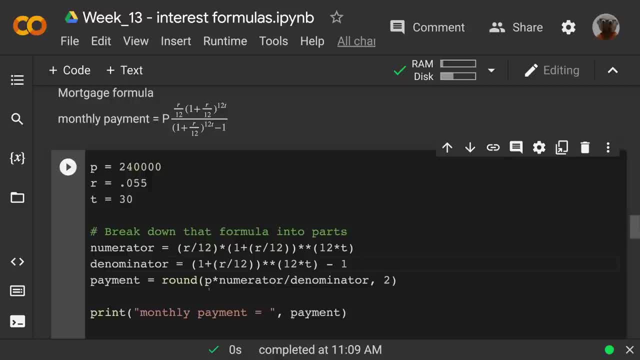 P times numerator divided by denominator. So there's my mortgage payment. So P times numerator divided by denominator. And then I'm going to round that because that's going to be a very long decimal. I'm going to round that, So it takes the first argument and then the second one: how many decimal places? 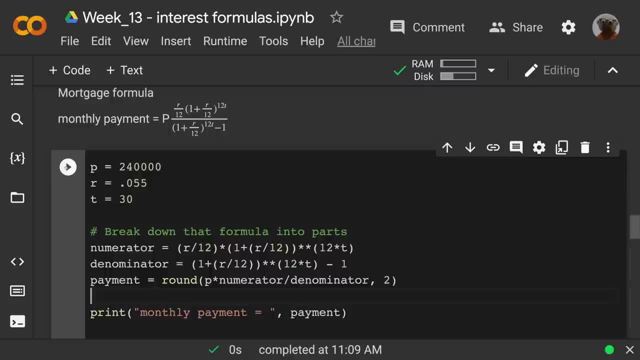 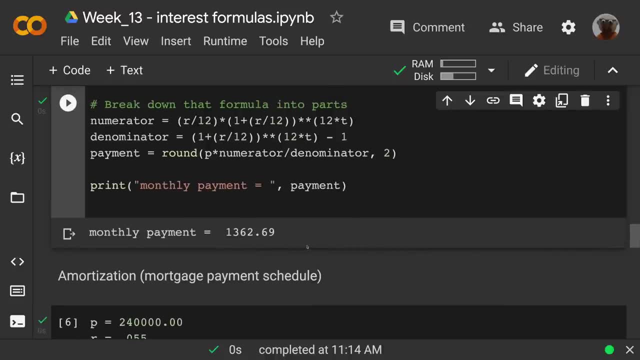 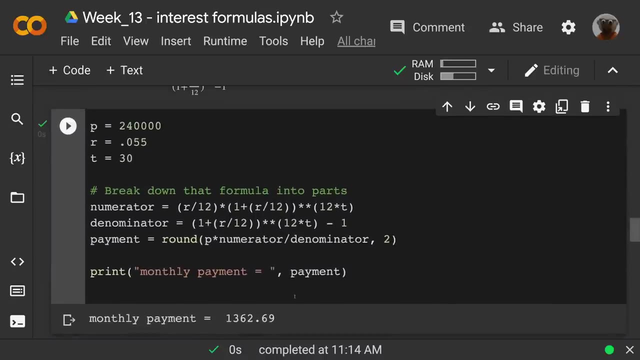 There we go. So when we take a look at this and when we run it, Mortgage payment 1362.. And 69 cents. So given that, then we know that's the payment that will make this work out, That after 360 payments of this, 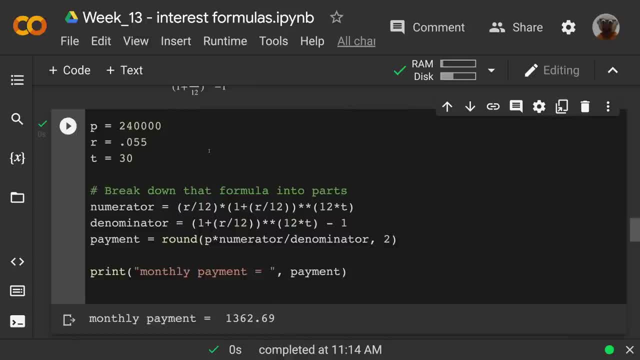 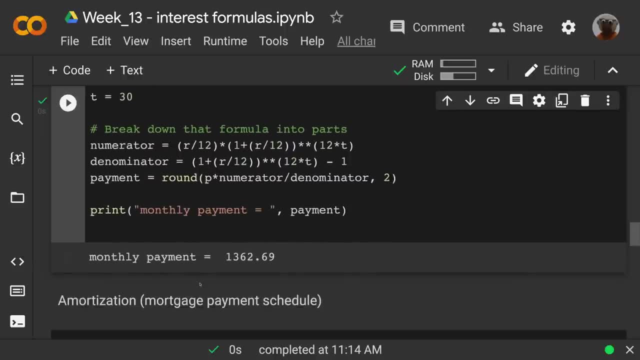 So each time you know we're still accruing interest and we're still making a payment, and it's going to work out now to see how that plays out. We call it the amortization schedule. So and that's it. that's the mortgage payment schedule. And yes, all of these have the word more in it, which means death. you know, kind of like you know what's true in life. you know death and taxes and, I guess, mortgage. But yeah, it was very morbid when people first came up with this word, but it stuck. 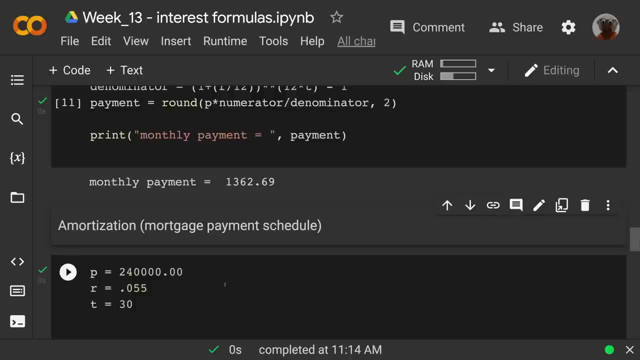 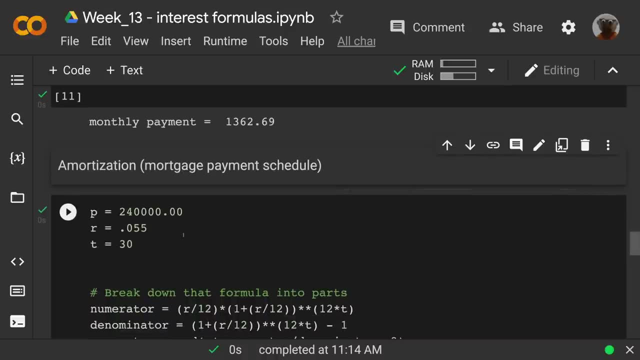 We will end this after this with something much more positive. So, don't worry, I don't want to leave you in the more morbid state. So the mortgage payment schedule. if I take this, there we go. given these three things. 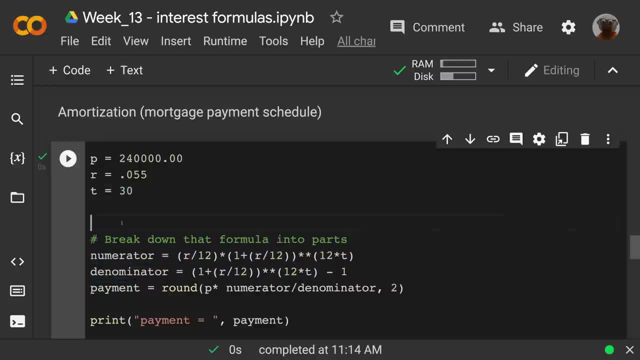 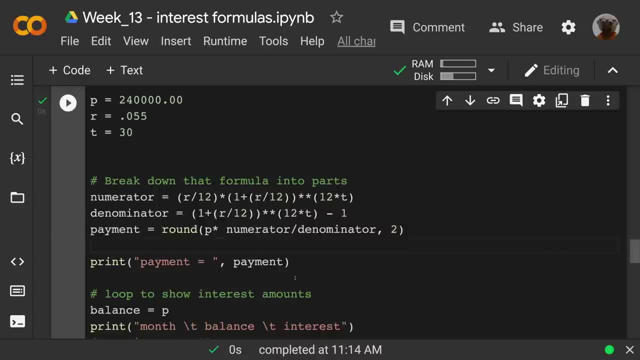 I just rewrote. I just rewrote all of this: how we're going to calculate the payment. All right, So I'm going to print this payment just like we did before. So that's all the same as what we just did. 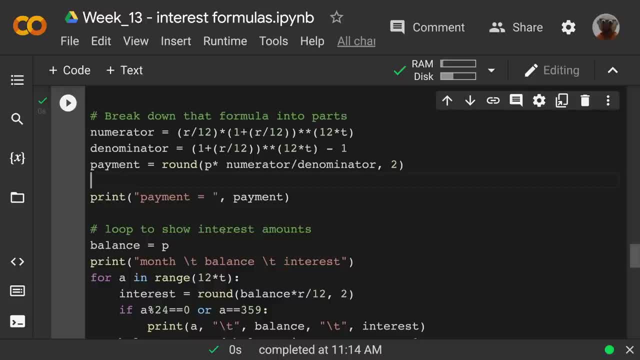 But the amortization schedule is. I want to have a loop to show the interest amounts, And we can also do this in a spreadsheet. That's pretty common And later on in the course we'll talk about that. So I can, I'm going to have a loop. 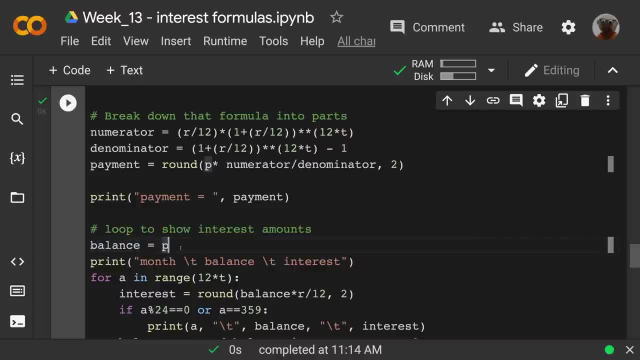 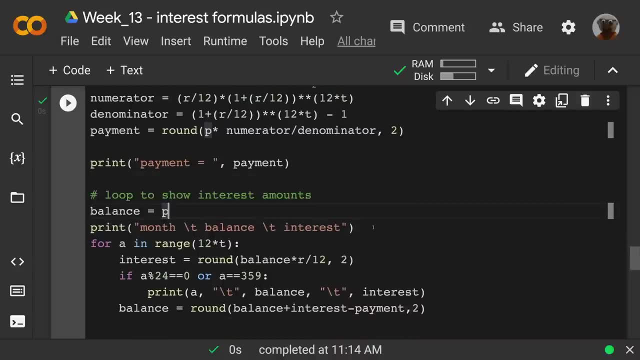 So I'm going to set this new variable called balance, and the starting balance is going to be that original P principle. Okay, Then I'm going to print this, which is going to be my headings month: I'm going to put a tab there, balance, put a tab and then interest. 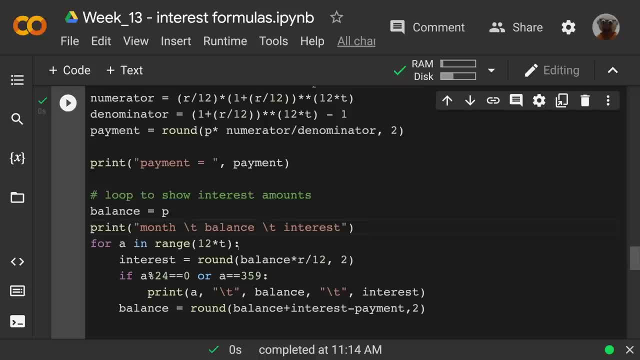 So that's what I want. I want the number. you know what month am I talking about. I'm going to put a tab there, balance, put a tab and then interest. So that's what I want. I want the number. you know what month am I talking about. 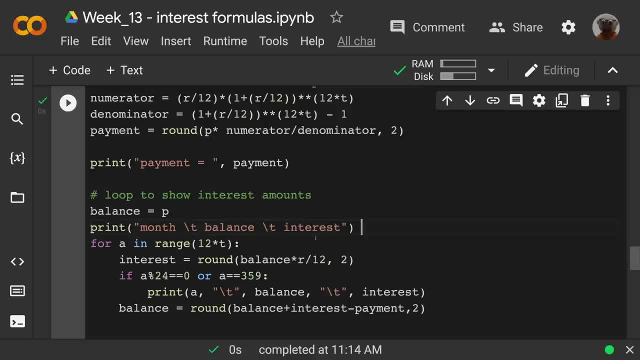 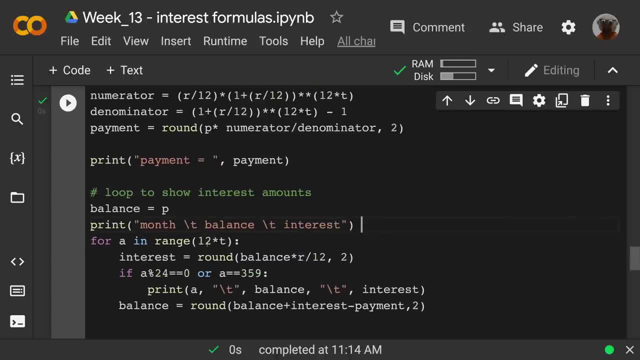 I'm going to put a tab there. balance, put a tab and then interest. What's the balance at that point? What's the balance at that point And then what's the interest that I'm paying for that month. So here's what we have in my loop for a and range and how many months. 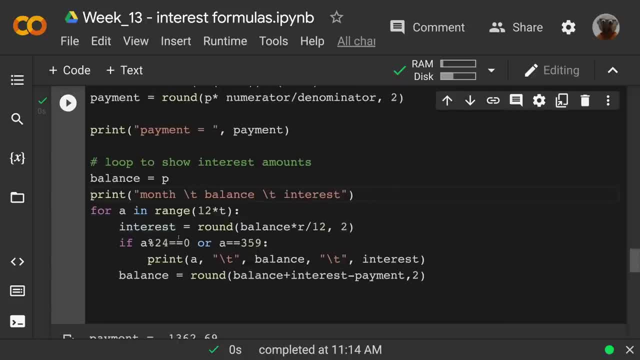 12 T. Okay, So the interest um is round. So again I'm going to round these, because calculating these you know it's going to be a lot of we're decimals. I want it to be two decimals: dollars and cents. 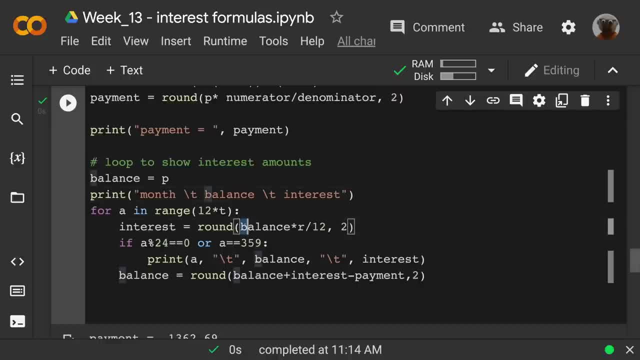 So the interest that we're going to pay is- this is simple interest again- because that short term, this is only for one month and then we're going to manually compound it here in this loop. So I do want simple interest. 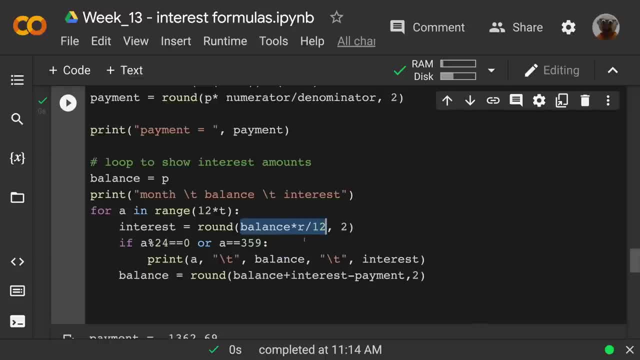 It still has usefulness: Balance times. so that's my P for that month. times R and then T is 1- twelfth. So I'm not just going to multiply by 1, I'm just going to divide by 12.. 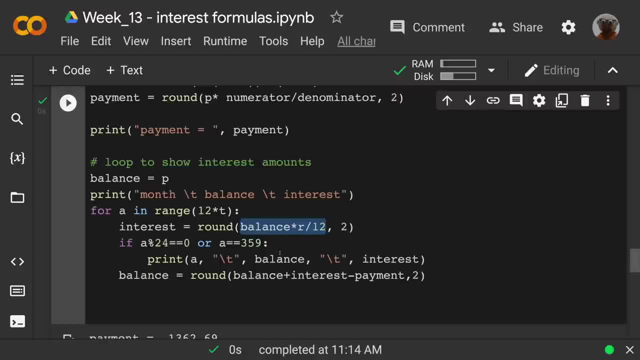 But that's what it is. this is the original simple interest PRT. the balance is the principal for that month rate, and then time is 1 twelfth. so I'm just going to divide by 12.. So there we go. 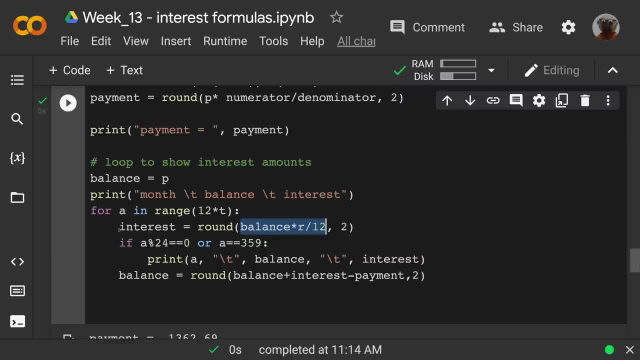 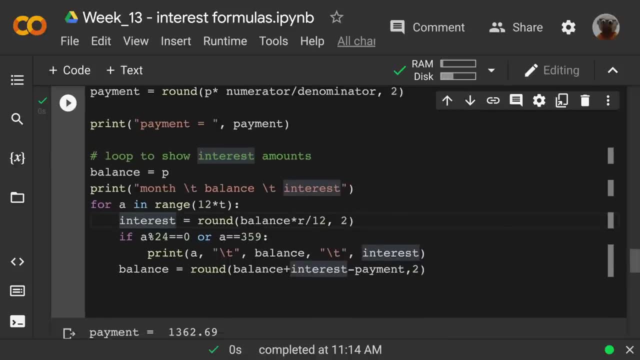 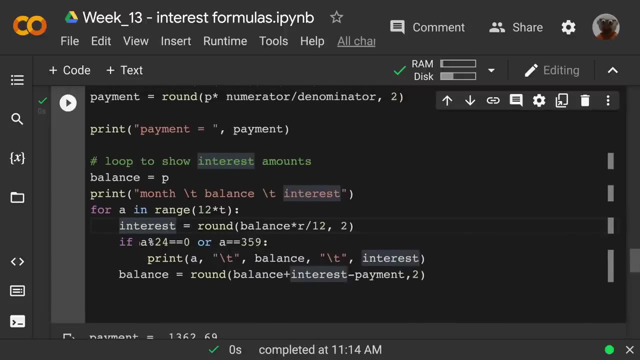 And all that. I'm going to round it to two decimal places. So now that I have the interest, this will still calculate. the interest- and I just put this here for the sake of the displaying- is that I only want Now, if A is divisible by 24, you see, remember the modulus A divided by 24, if the remainder, 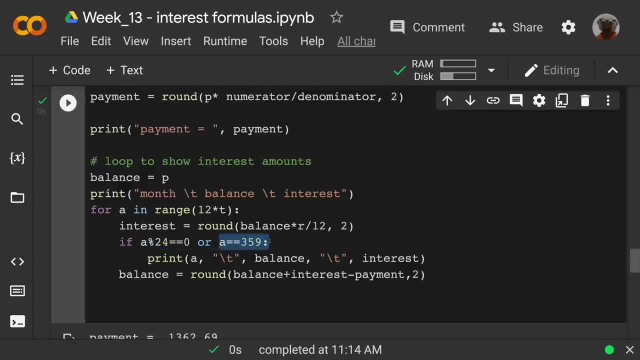 is 0, then, or if A is 359,, which is going to be almost the last month. So these are the ones. so rather than print out every single month, I just want to skip a few. Normally, if I put this in a spreadsheet, I'd want the whole schedule and I'd print. 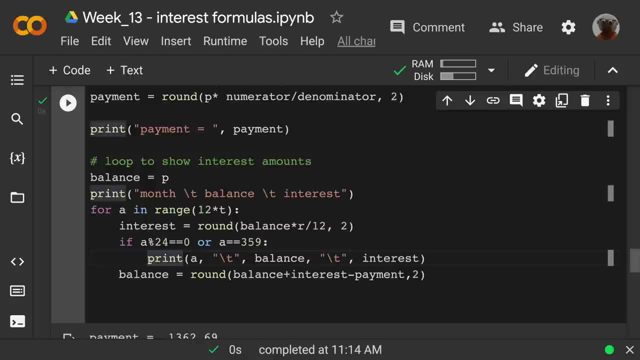 out all 360 months, Only for these. we're going to print out a select few. So I want A and then tab, so that you know A is going to be what month, because that's A in range, and then tab, balance, tab and then interest. 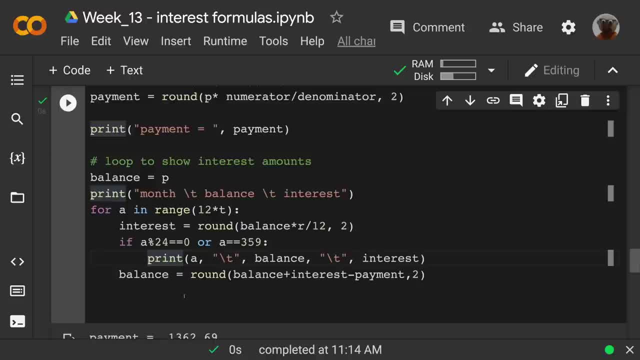 So there we go. That's what's going to line up month balance interest. So then, after I do this- so I put this line last, Because the first time through I want it to be the current amount, and then I'm going. 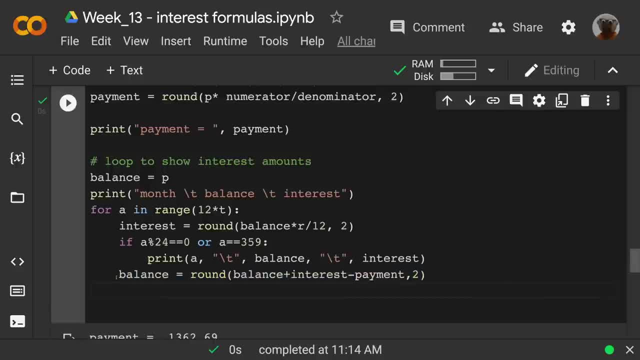 to increase the balance. So you see what I'm doing: to increase the balance here. Alright, I'm going to round balance plus interest, minus payment. So you see that's what's happening every month. So we're manually compounding it. 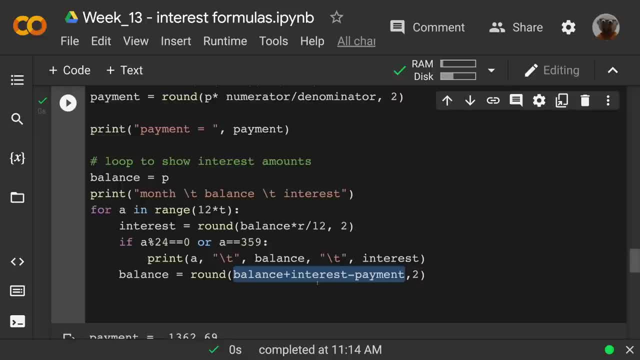 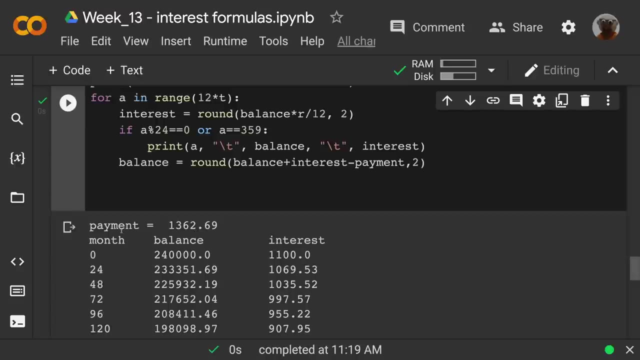 The balance at that month plus the interest that accrues that month, minus the payment, And then round it to two decimal places. So when we run this, so we have the payment, it's $1,362, just so we can figure. and then 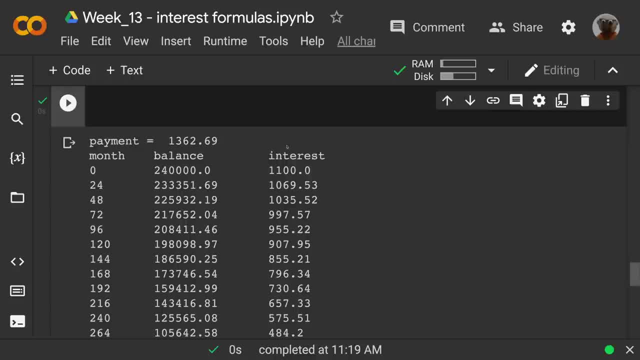 here we have our abbreviated table: month balance interest, So month zero. we start out owing $240,000, as we expected. But look at that. This is why it makes a difference. You're paying $1,100 in interest. 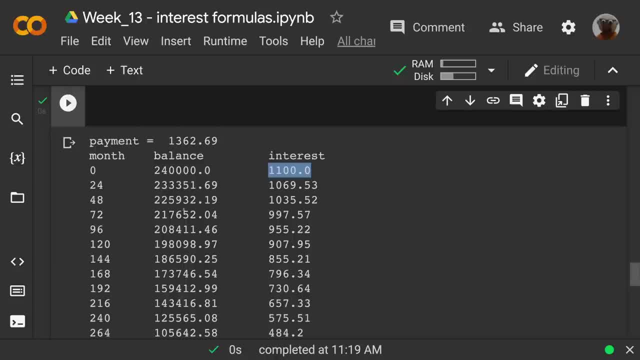 Just for that month. That's a lot of money And you know that's it, It's, you know it's almost the whole mortgage payment. You know it's shocking at first. after you do this enough times, you come to terms with. 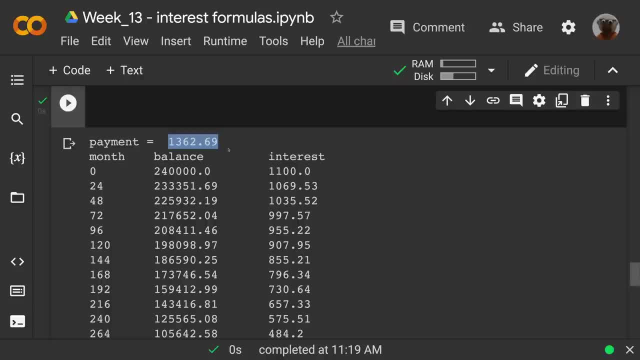 it and say, yes, that's right, I'm paying almost all interest at the beginning, you know. And then $1,362, pay $1,100.. So really then notice that only $262.. $262 is going toward the payment. 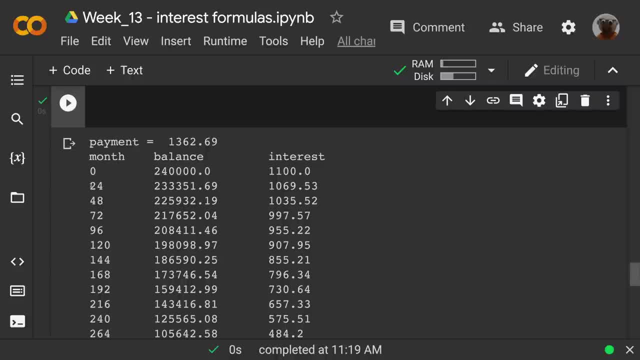 Now we could see this really increase slightly, but at month 24, we've paid down some things, But it's probably not as low as you'd expect it to be. You'd think like, oh, I'm paying so much, I'd expect this balance to be lower. But you see, you really just chip away at it And even then you're paying less interest, but it's still more than $1,000.. And that's, you know, month 24, so after two years. 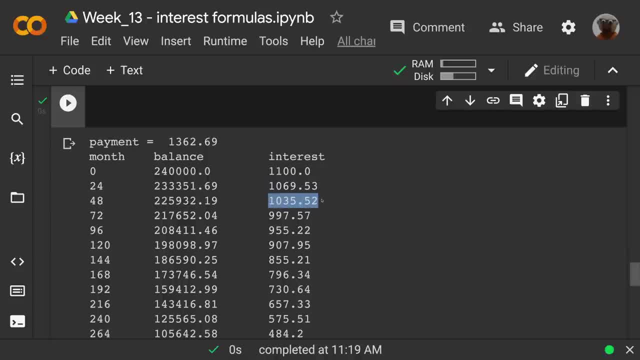 And you see you're paying less interest, but it's still more than $1,000.. After month 48, you're paying a little bit less interest. We do see this moving in the right direction. You're paying this down and you're paying a little bit less interest, but probably not. 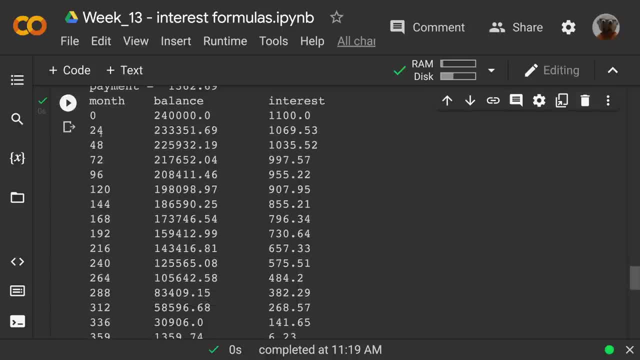 going down as quickly as you'd want And that's why I just wanted to skip ahead. You know, every two years we check in and see the balance and you know how much interest we're paying. You know we take a look at this. 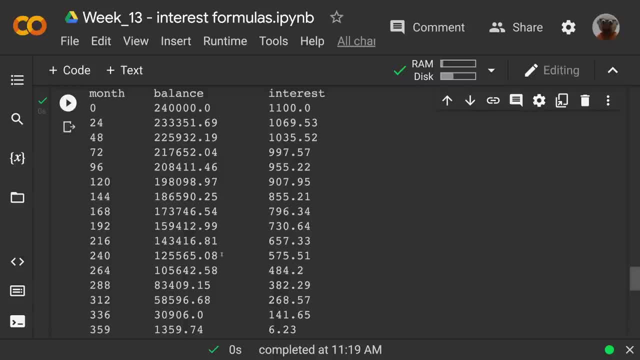 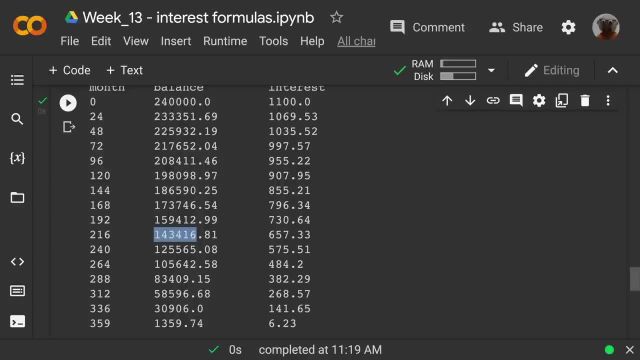 Now you know, we take a look at this And we look at this. So if we have just over $140,000.. So remember, we originally borrowed $240,000, still owe $140,000. But at this point, now that difference, we start building annuity or start building. equity in. you know, if this is a mortgage equity in the house, which means the house is worth a lot more than what we owe, And so you could borrow money against that. You know, home equity loans, that's where that comes in. 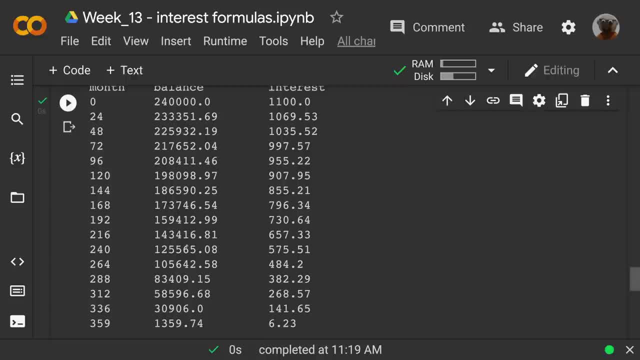 As you start getting lower and you know the value of the house is worth a certain amount and then you only owe a certain amount. the difference you know. you can actually borrow money against that. That'll be a discussion for another time. 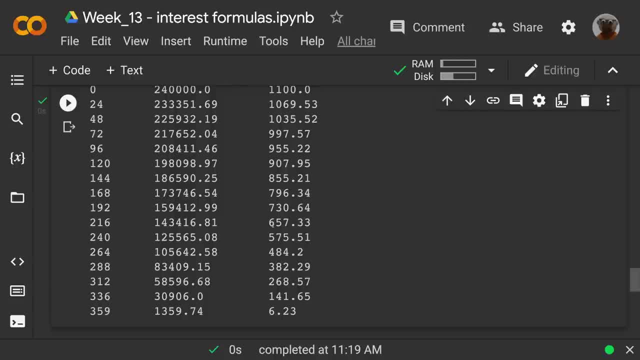 So we have this And finally, now it's still a lot, I mean, you know, sometimes it's, you know, to think about: wow, I'm still. you know, look at that, 20 years in, I'm still paying more than $500 a month, just in interest. 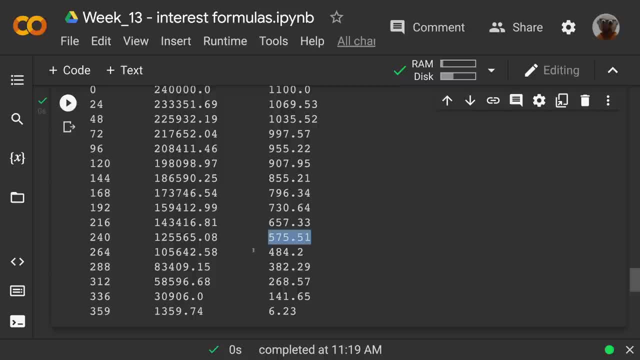 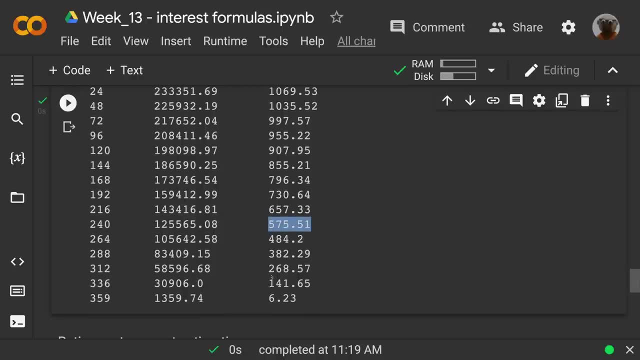 You know, but at least that's only $500 a month And you know we're getting the vast majority of our payments are going at this point to paying off the mortgage. And now when we take a look, you know, look at that- double digits instead of three digits. 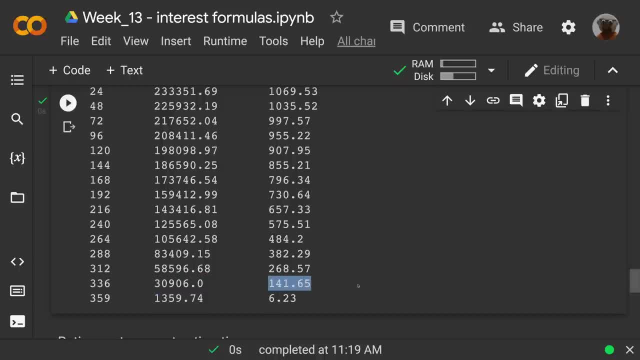 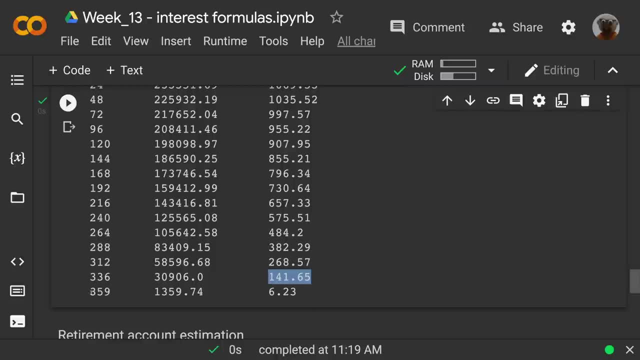 $30,000.. And then the amount of interest at that point is $140,000.. So I wanted to skip ahead and then just do month 359, because look at that Now, the balance at that point is just under what the mortgage payment would be. 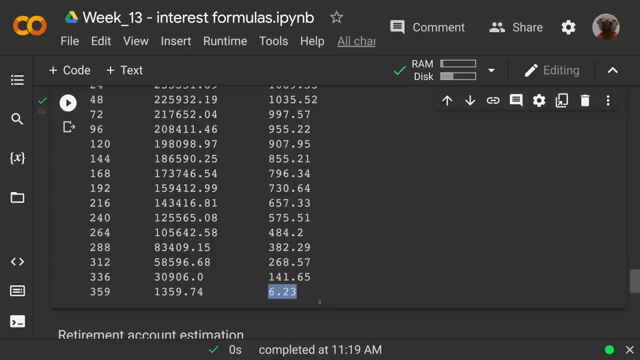 And then the interest is this tiny amount- And that would be, if you know, month 360, when you make your last payment it ends up being like $4 or $5 more than the mortgage Normal mortgage payment. 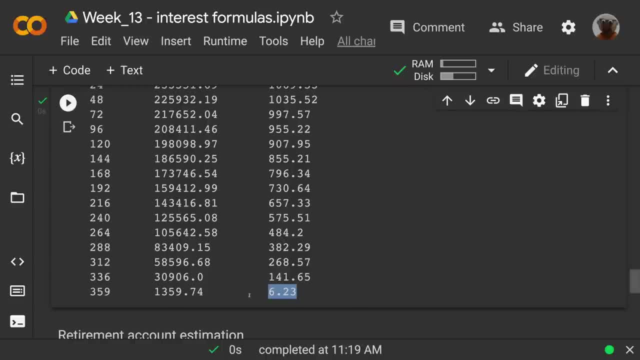 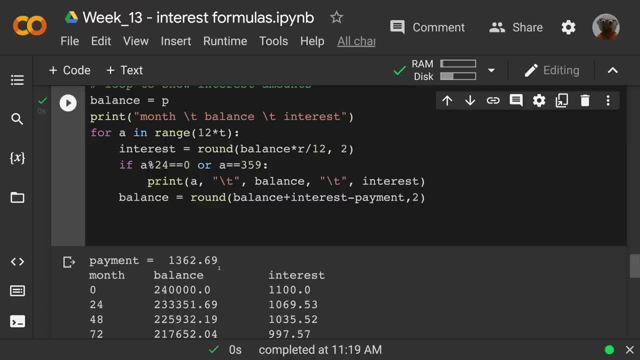 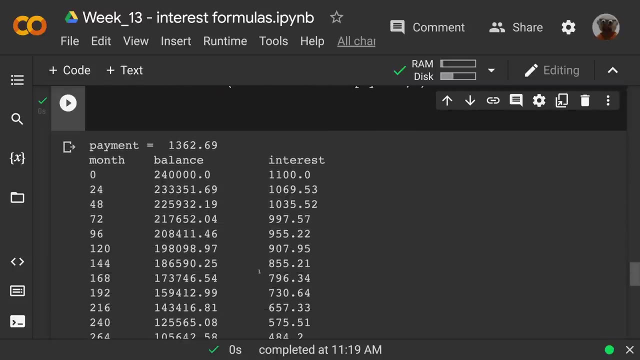 But then it's done. So it works out that that monthly payment, you know, using that formula, gave us that monthly payment $13.62 and $0.69.. And that monthly payment did work out that that exact payment. as you know, we're look. 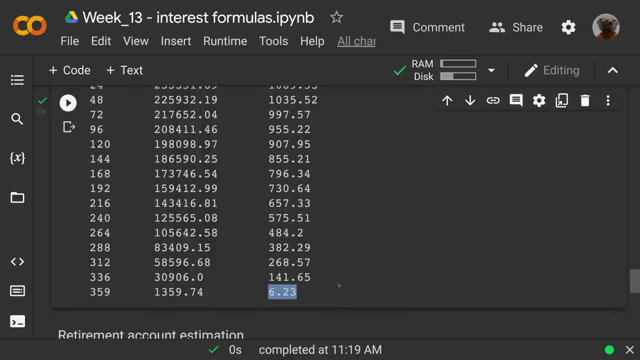 at the amortization table at 360 months it was, you know. we paid it off And there we go For an extra $5. The last month, I'm not going to stress about that. So these are, you know, interesting things to think about, seeing how, using these percent. 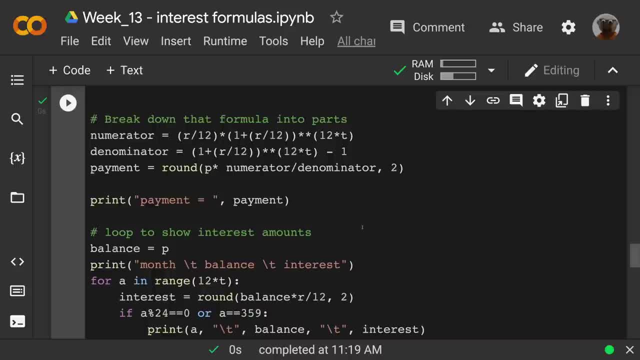 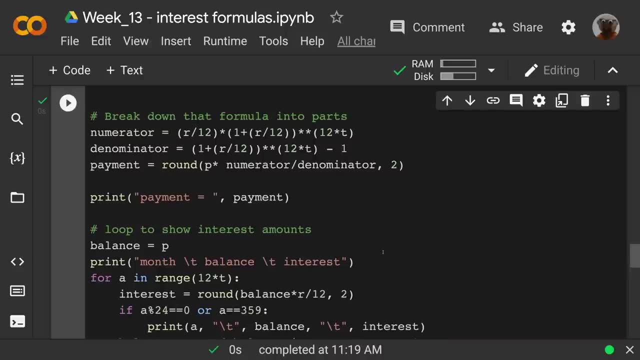 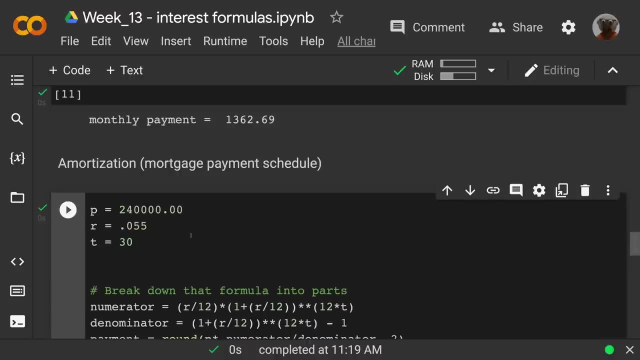 interest payments applied to loans, how that plays out, how you're paying off interest, how we're making use of the simple interest and then paying down this balance. So this mortgage is the most common but for any large amount of money over a significant 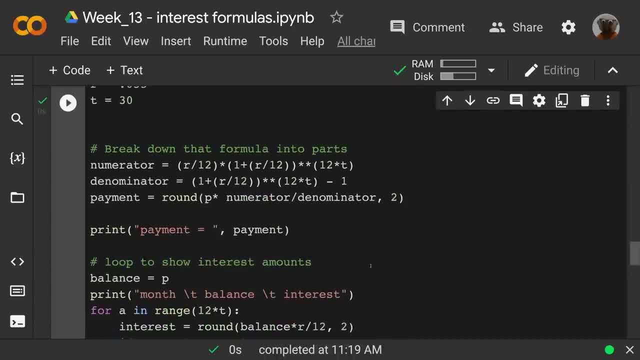 amount of time we would use this formula. It does not have to be a mortgage, Car payments- not always, because a lot of times they're a lot lower. But if it was a car payment for, like, a particularly expensive car or that over a 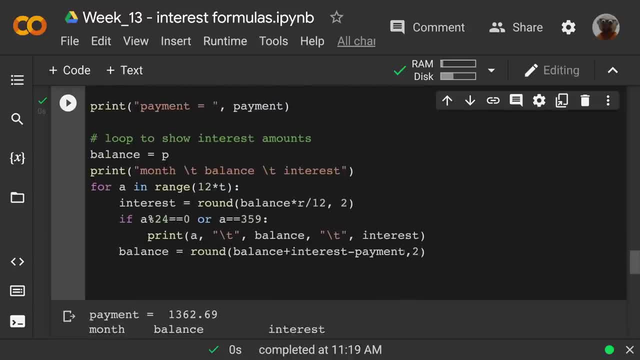 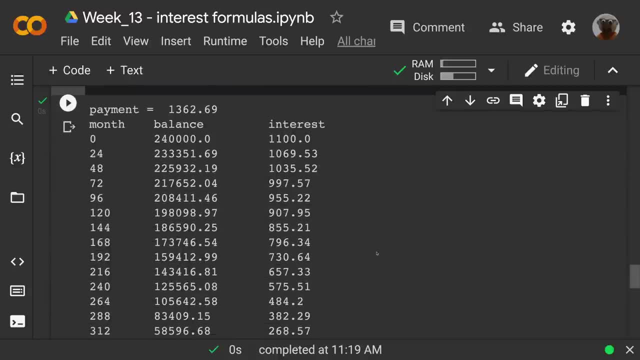 longer period of time, then we might use this. It doesn't have to go to 30 years, That time can be anything. So we see this, you know paying off this debt over time. So let's use something very similar. 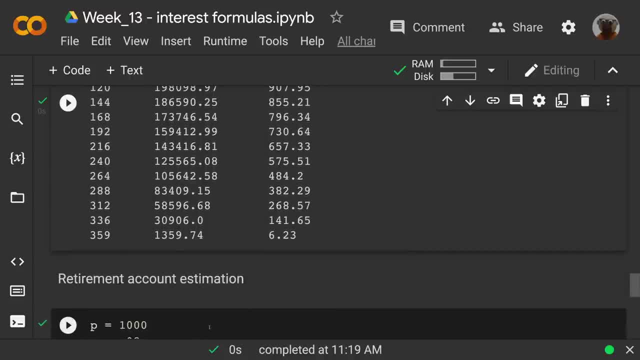 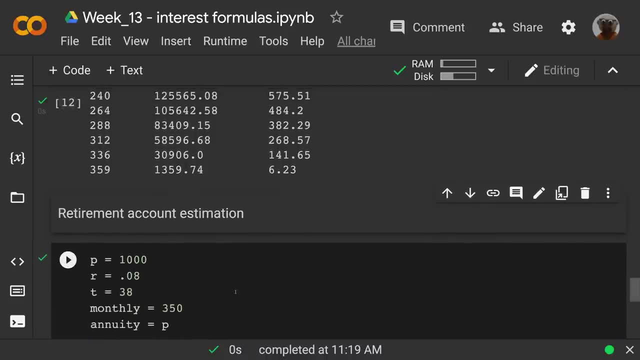 But let's talk, Let's turn it around and have something positive. Retirement account estimation- Now this one, instead of owing money- you know, this P is not money that I'm borrowing, It's money that I'm going to put into an account. 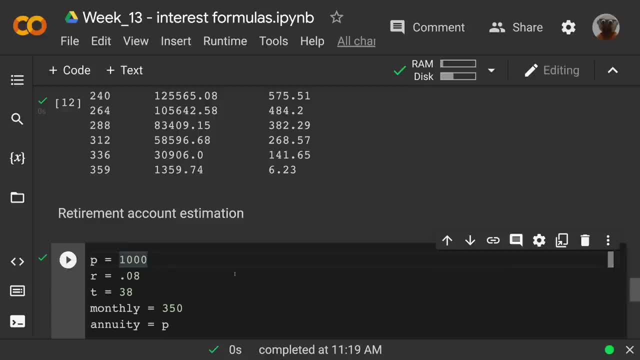 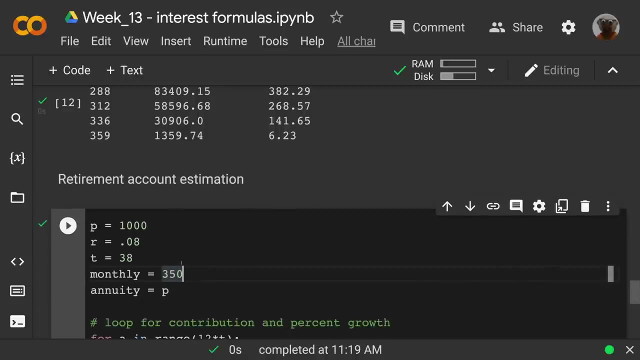 And instead of owing money every month, I'm going to contribute, And so there's no formula for this, that I'm just going to estimate this. Oh, okay, Let's say $350.. Just because You'll see how this plays out. 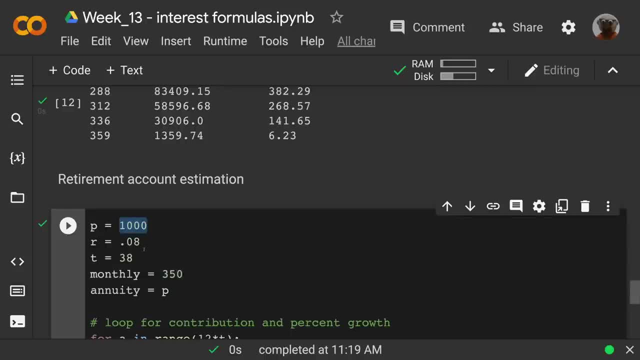 I just picked these numbers here. So let's say the principal is $1,000. And this is just estimation here. Well, let's say you start out with $1,000.. Now this is where the estimation comes in. 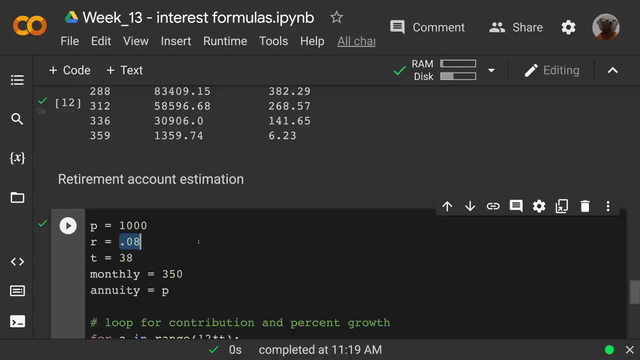 Most of the time a retirement account. you know any decent fund manager is going to be able to get you 0.8% or 8% interest. So now this is your money growing in an account. this isn't you paying off a debt, it's your money. 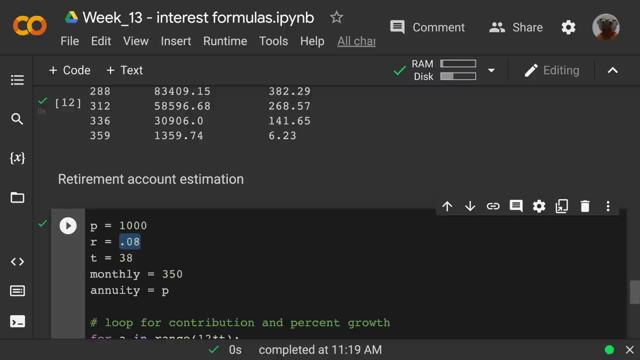 growing in an account. so if you had a thousand dollars and we estimate that it's growing at eight percent per year, that's great. and i made this time 38 years, as you know, not entirely random. it was. i just thought, like age 22 till age 60, um 38 years. so you start it, put a thousand dollars. 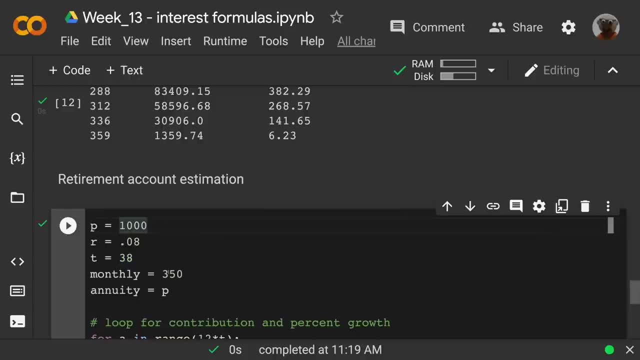 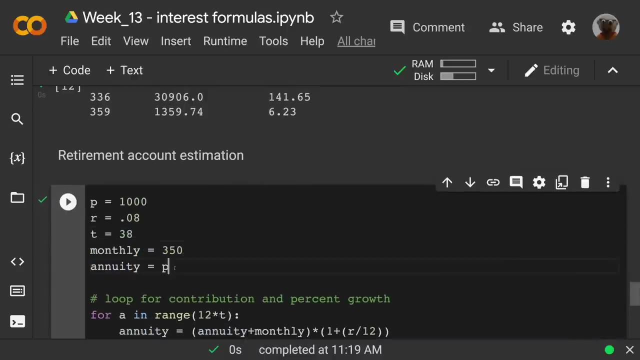 in this account and then you start um saving that you know from that point, like you know your whole career. you put away 350 every month in this account. okay, and i'm going to establish this other variable, annuity, which i'm going to start out. the original was p. 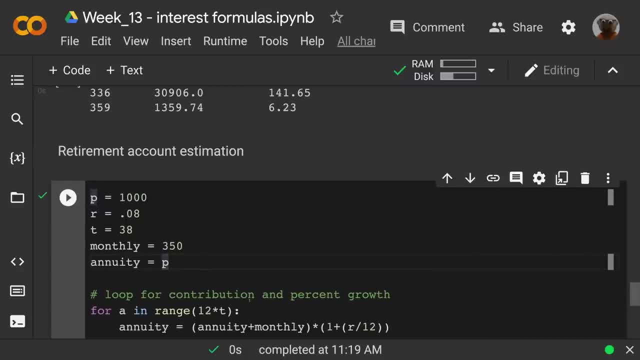 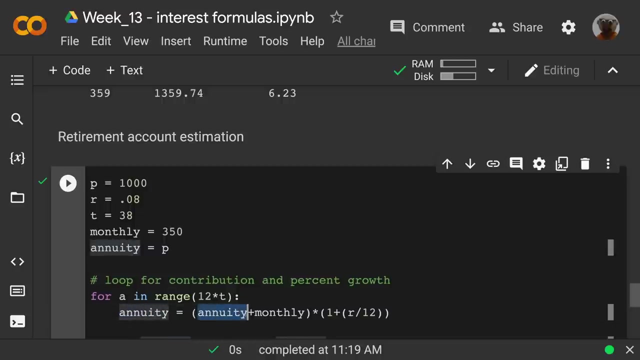 so now here's my loop for the contribution and the percent growth. so again 38 years, so for a in range 12 t. so there you go, because every month we're contributing something. so notice what we're doing with this annuity: we're taking the annuity that we already have. 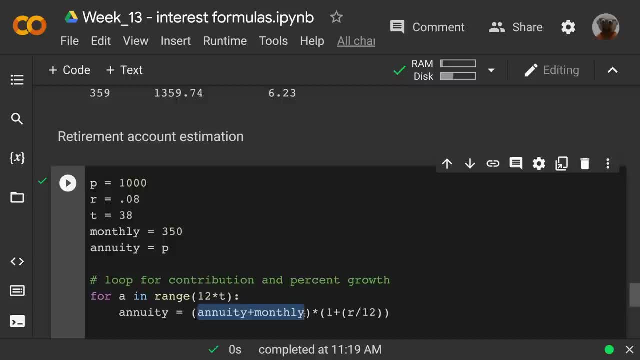 plus the monthly contribution and then that's going to grow one plus r over 12, because that's a monthly contribution, and then that's going to grow. notice that percent increase formula. but this is monthly. so the exponent, if it was n, t, the exponent n would be 12 and t would be 112, which cancels out to one. 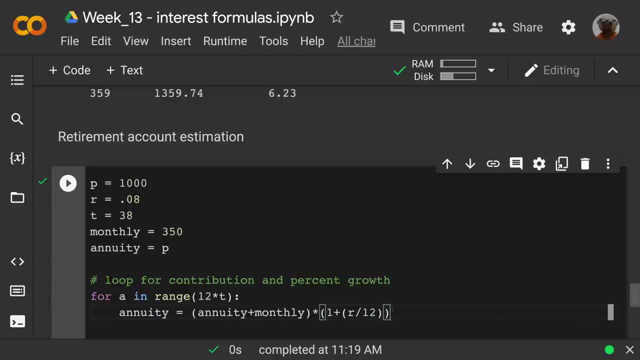 so i don't need to write the exponent of one, but that's where this comes from. it is that same formula, r over n to the n t, but n, t, n is n is 12, t is 1 over 12, and so that cancels out. 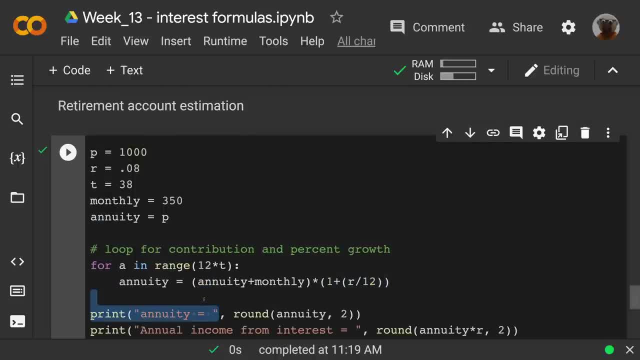 each month, then if we take this- and that's why i wanted to break this down, still monthly, because i want to allow for this contribution here, the annuity plus the monthly contribution, we want that to happen each time and then it's going to grow. so in this loop, now this continues. 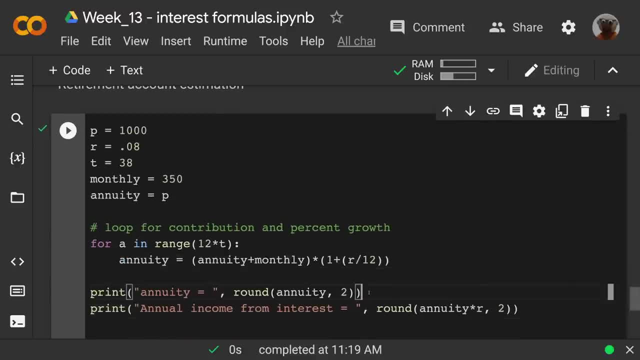 to grow. so at the end, we're going to print this out and i'm going to go around, because that'll end up being a weird decimal annuity. okay, so now the annuity is going to seem like a lot, but this is what we want. to break this down. if we're 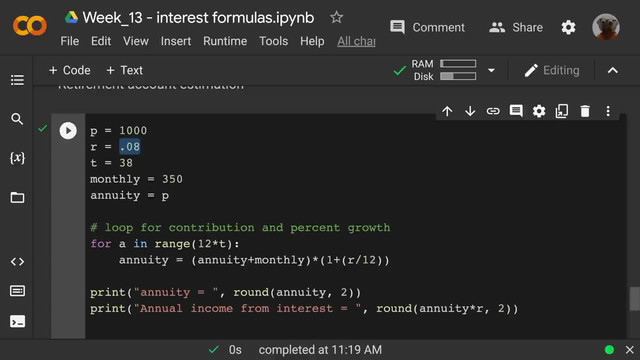 if our rate is eight percent, so at the end let's say it's still earning eight percent when you start taking what? so the annual income from interest, you see? and so that's annuity times the rate. that's it, and yeah, i'm going to two decimal places. 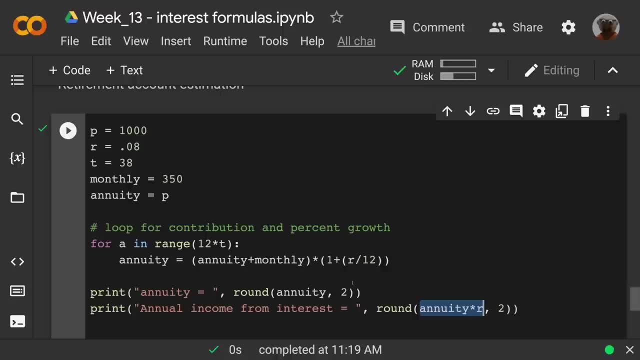 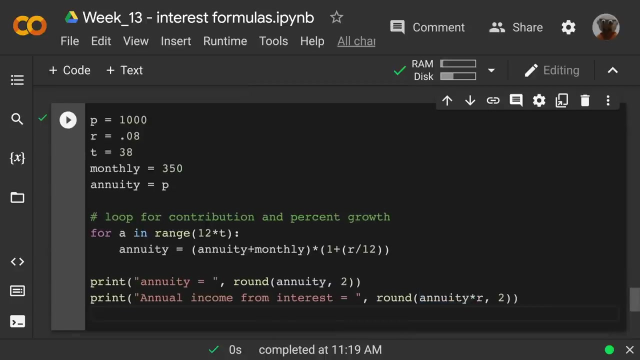 but that. so if i have this, um, this amount of money that i'm going to eventually get to, then the idea is that money now is yours in the bank, or in this, in this fund, somewhere, that the annual income is just that percentage rate. so when we run it, 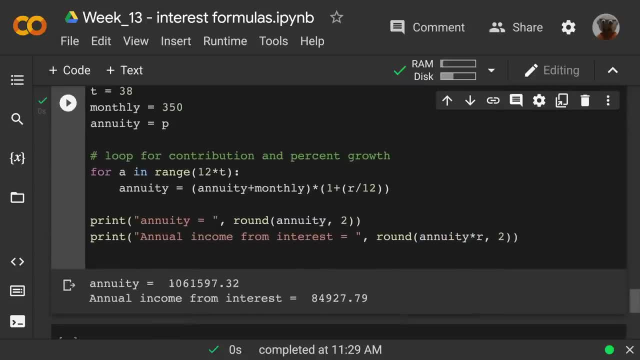 so take a look at this and you'll see that the annual income is just that percentage rate. you can take a look at this annuity here. so one zero, six, one five, nine, seven, yes, that's more than a million dollars, and if it continues to earn that, eight percent the annual income. 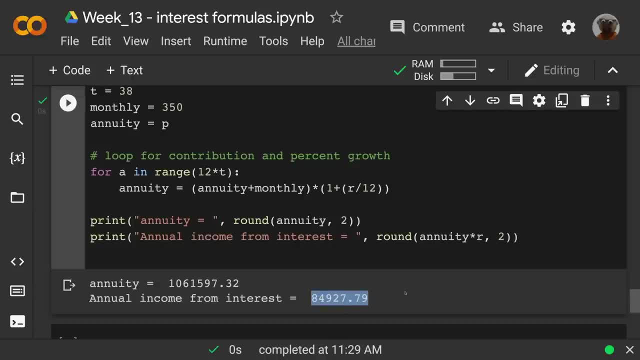 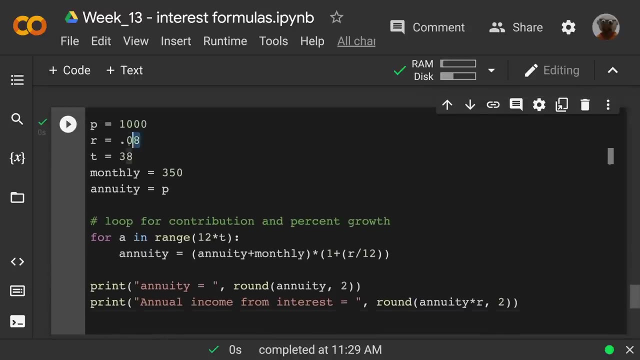 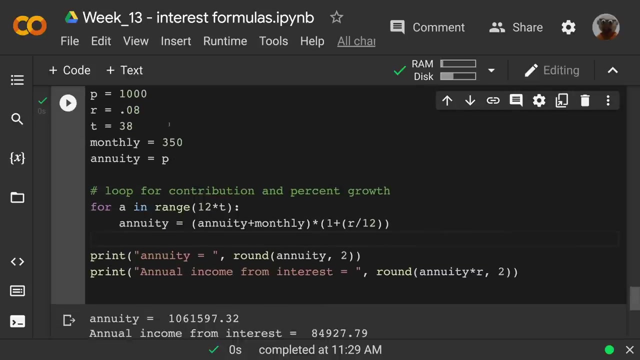 just from the interest is eighty-four thousand dollars or almost eighty-five thousand. and that's the idea that this money in the bank or in investment, not not in the bank, not saving, because nothing in the bank is going to get you this eight percent interest that makes this happen. but this retirement investment, if you're, you know you have. 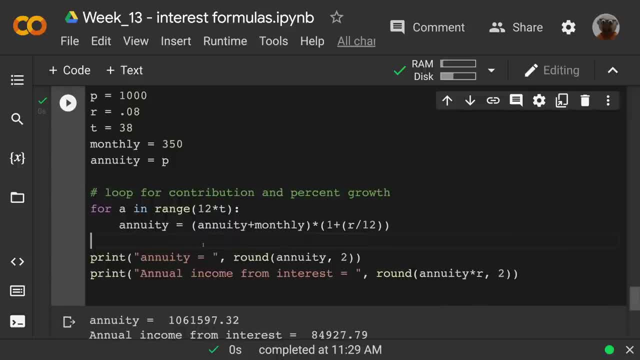 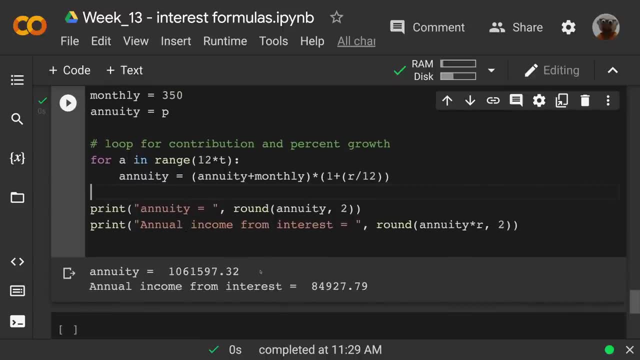 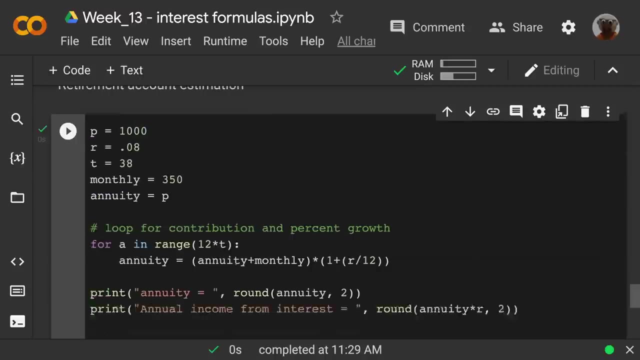 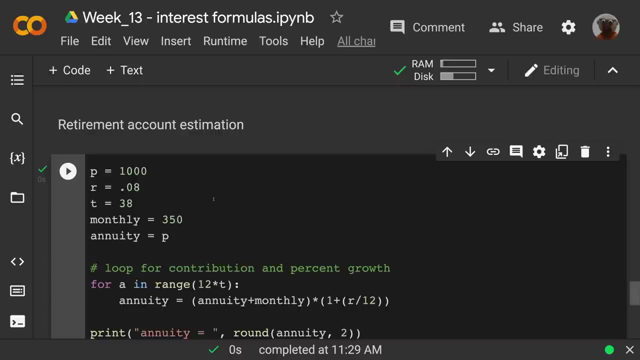 this and you can contribute something. it's you're constantly contributing and it's growing, so at some point then you retire and you have this million dollars that earns this amount of interest, and I just picked, you know, 38 years. the earlier you start, the better, and the later you start start. 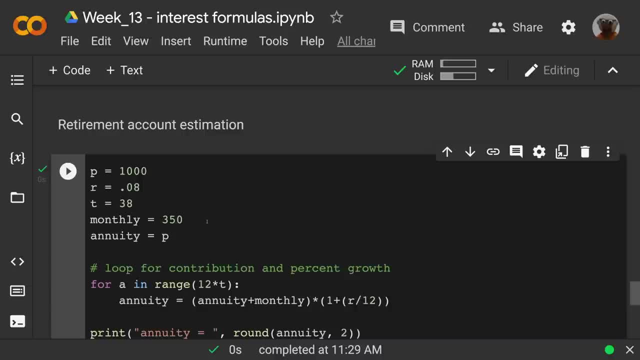 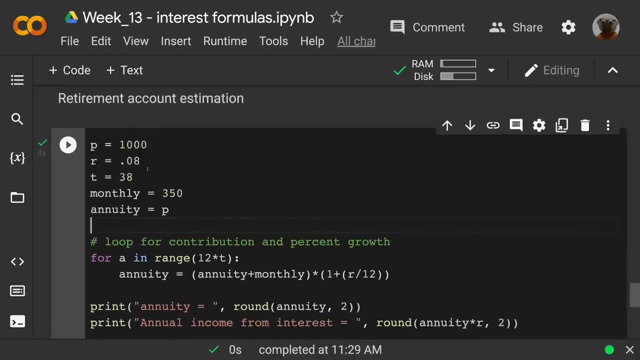 taking money out. you know it can grow even more that you could take the money out at um. you know, uh, age I just I just rough estimated did age 22 to 60. you know. You know, if you start as early as you can, I mean even 18 and you know, till 68, I mean, look at that, that'd be like 50 years. 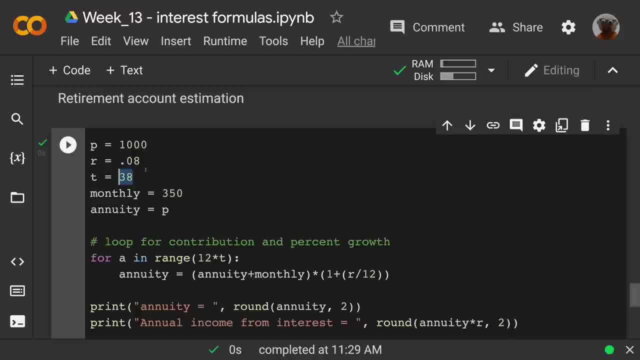 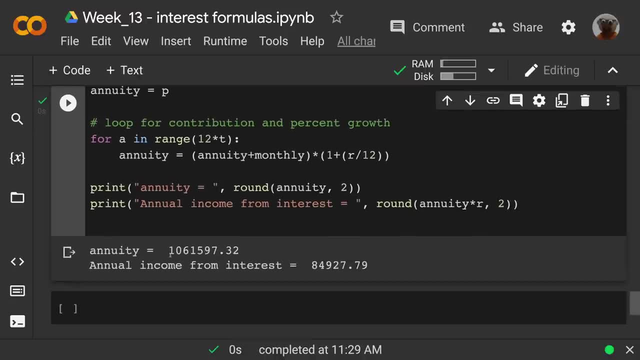 That really is what makes a difference, Because remember this snowball, so that 8% in those later years, that's 8% of larger and larger amounts of money, And then if you get it to this million, then 8% of a million is more than $80,000. 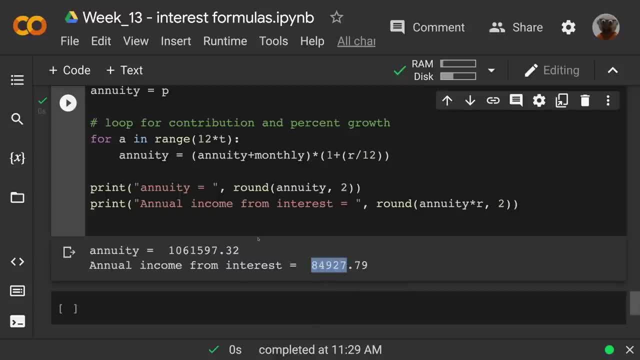 So that's the idea. We want to get to this larger amount of money that just the interest on that. you know, if this investment keeps going, just the interest on that is enough to live on And you take the interest and then you're back to this amount which will earn interest the next year. 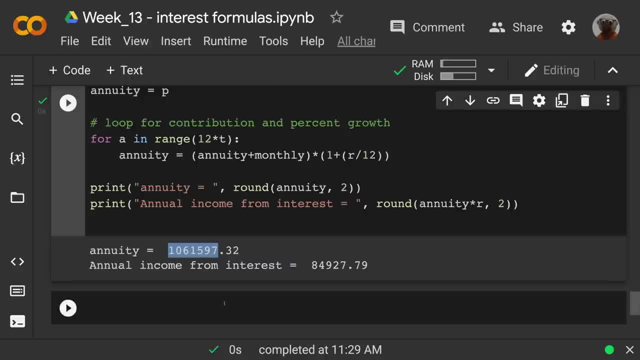 So I'll leave you with that positive idea of how we can use all this. You know that's what I want. Use all these you know percent increase formulas. Use all these you know percent increase formulas to. you know, turn that into money in the bank. 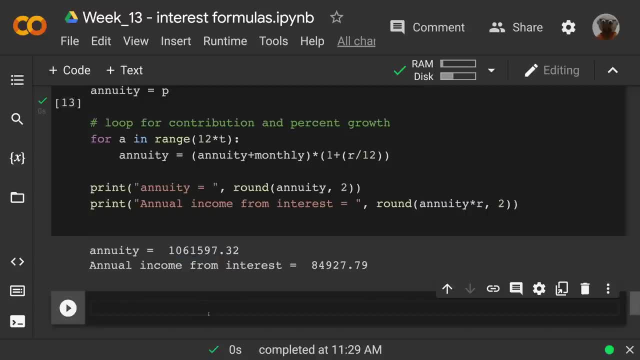 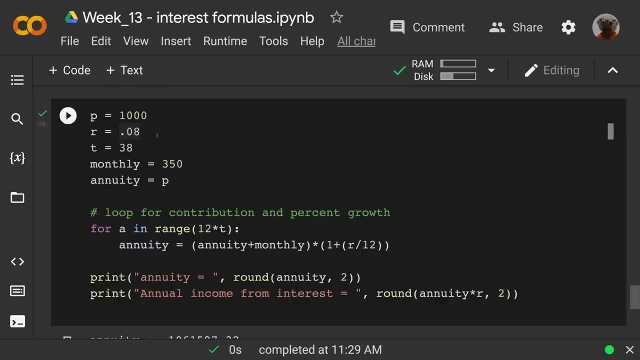 That's the goal here, All right, And you know, hopefully then it works out. And if you have this code, you can tinker with this and say: you know how much do you start out with? You know, keep this rate, maybe change the rate a little bit. 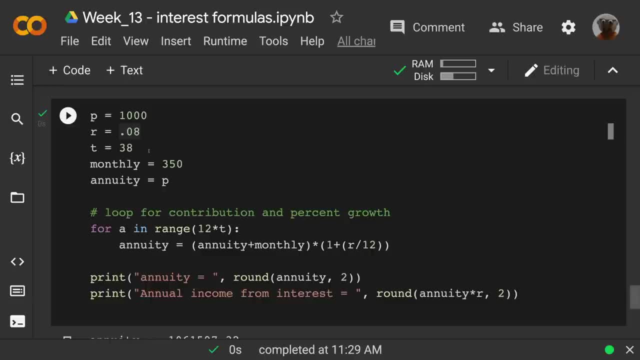 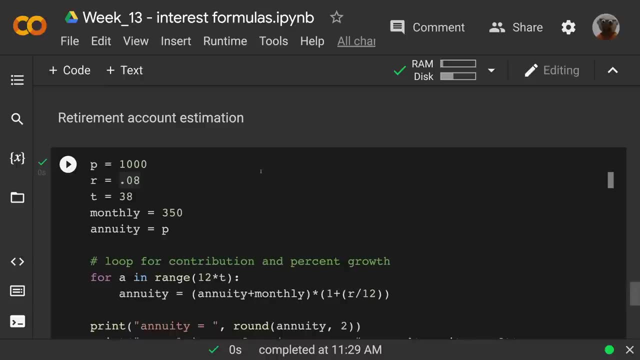 Oh, you know my fund manager is doing really well: Change the time, monthly contribution, You can tinker with these and run it and you know see the results. So you know prepare for, You know what you need to do to invest for retirement. 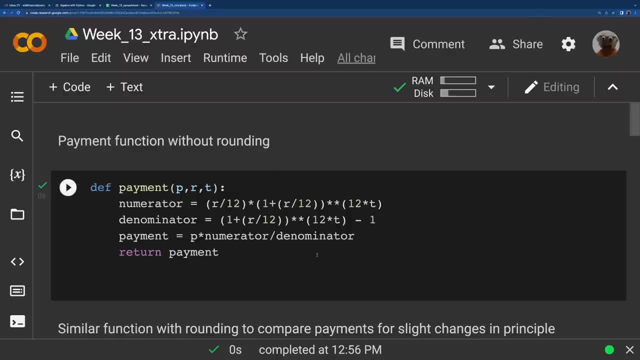 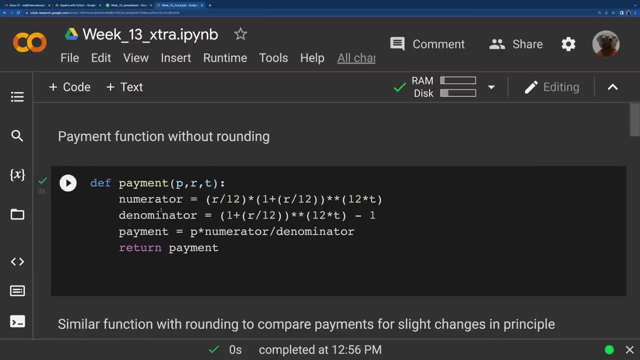 So let's look at some more ways you can use these mortgage formulas here. Now, like we were doing before, I'm going to define actually the payment formula as its own function. So there we go, And then payment, And I'm going to take the arguments P, R and T, run it through this formula and I'll just return the payment. 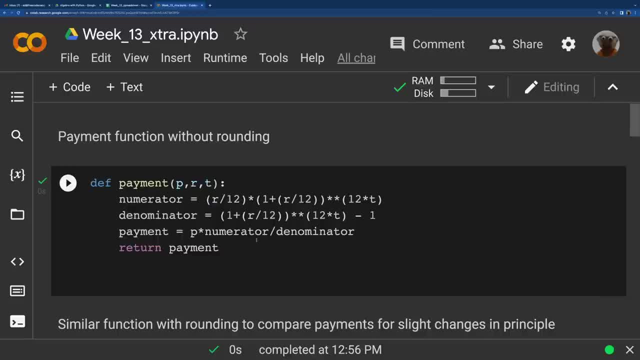 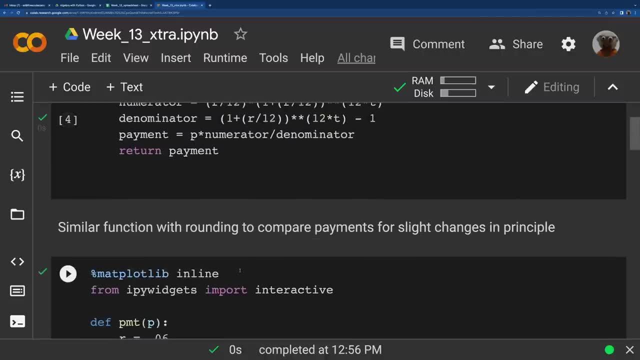 So this: you'll see some places we can use this And all of these. you know we're going to apply these to you know. let's say you know you're looking for a house, you're comparing different things. 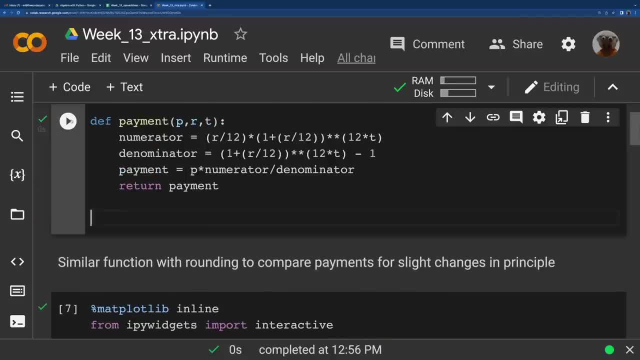 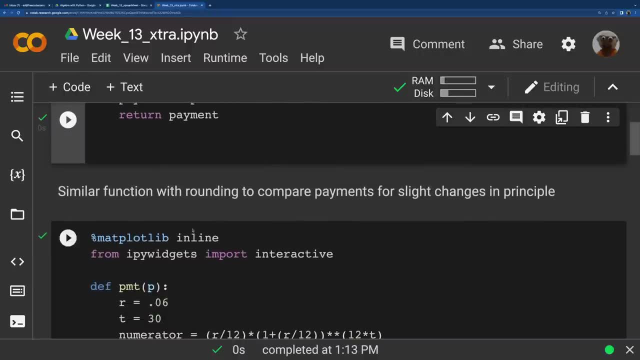 So to get this, I'm just going to run this And there we go, And I don't need to run that again. Now I have that formula here, So I'm going to do a similar function and I get something different. 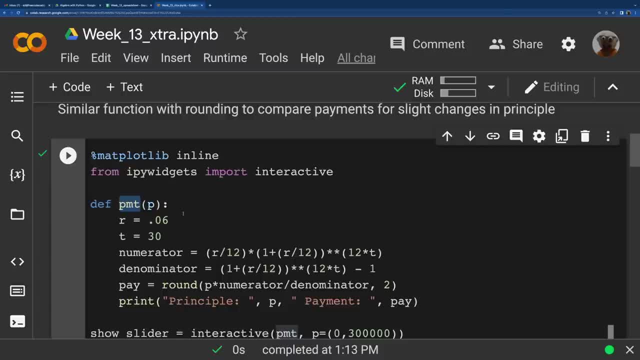 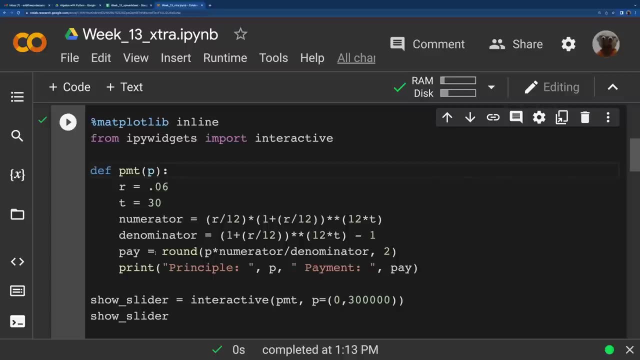 Because I just want to show you this one. I'm just going to define it PMT And I'm only taking the principal as the argument, Because I'm going to just give a set rate and time, So with this, and then I'll run that through, taking the input as whatever the principal is. 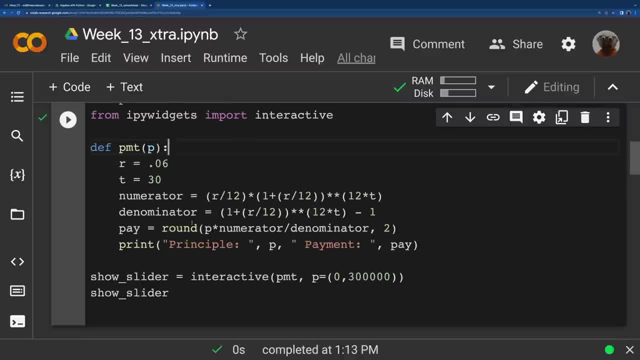 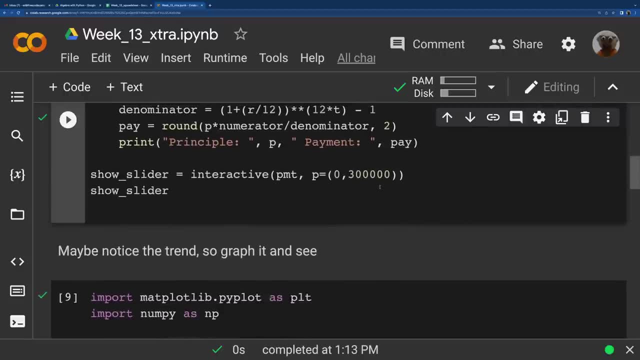 I'm going to calculate the payment And the reason why I'm doing this and we see these imports, is because I'm going to make this a slider Where I'm just going to Go from zero to $300,000. And see how the payment changes based on that principal. 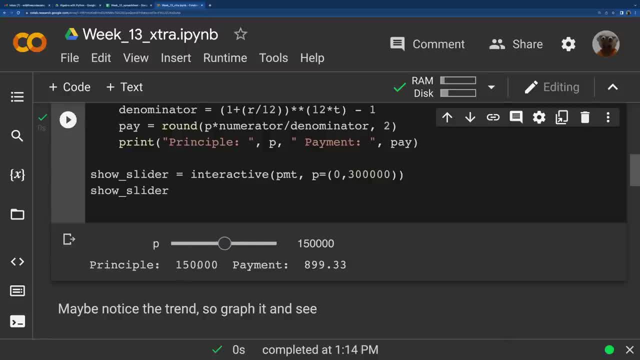 Of course the slider shows it's somewhere in the middle. For $150,000, the monthly payment would be $899.33.. And we can see how this goes up. And here's something you can do. You know. again, if you're comparing different mortgages or houses, you can see how does this really affect my monthly payment. 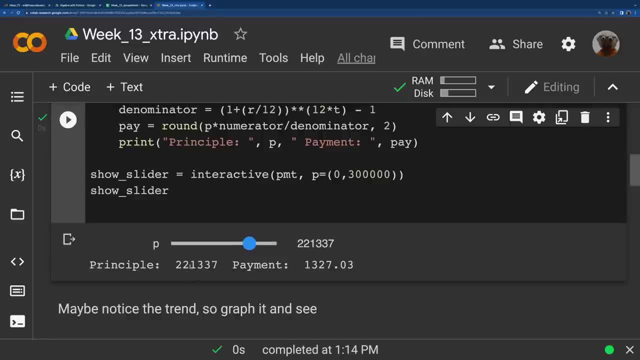 You know, And we look at this: Oh, $221,000.. Should I buy a house that's more expensive? I know my payment will go up, But the question is by how much? You see, And we can look at this, 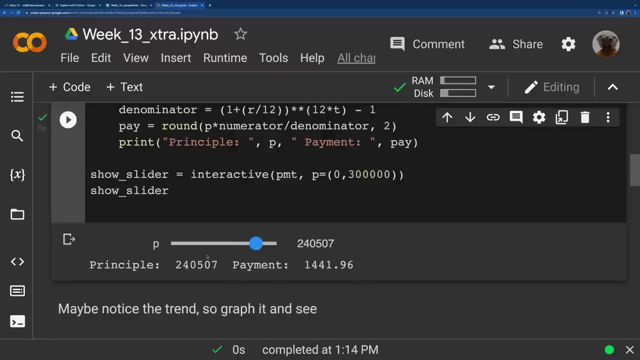 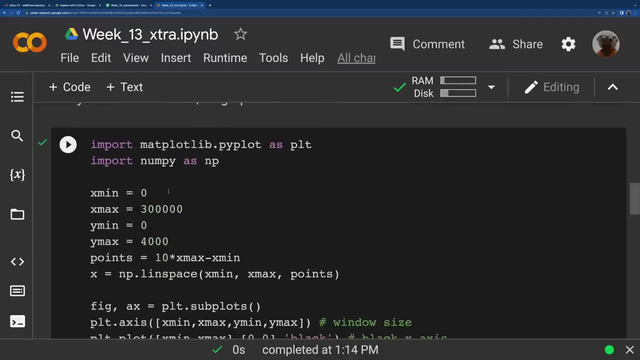 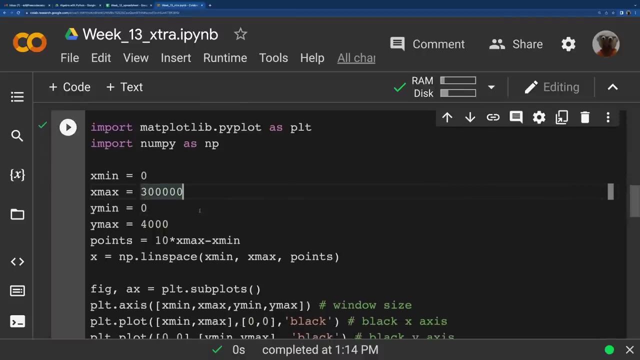 Now, that's great to see these exact numbers, But maybe I want to see the trend, Maybe I want to graph it. So notice our standard for graphing, And in this case I just define my X maximum as $300,000.. 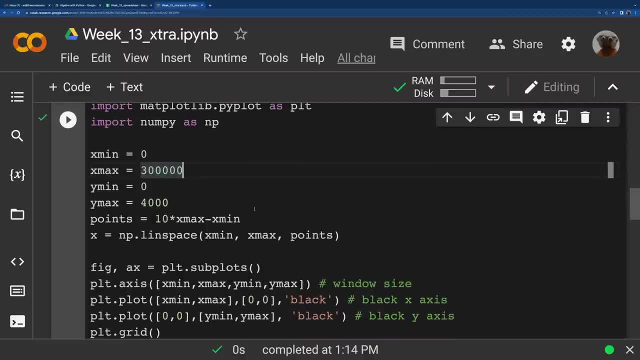 And my Y maximum $4,000.. That's going to be plenty, All these standard things you would already have set up. You know X min max, The points you're going to use for nplinspace And everything you're going to do to graph. 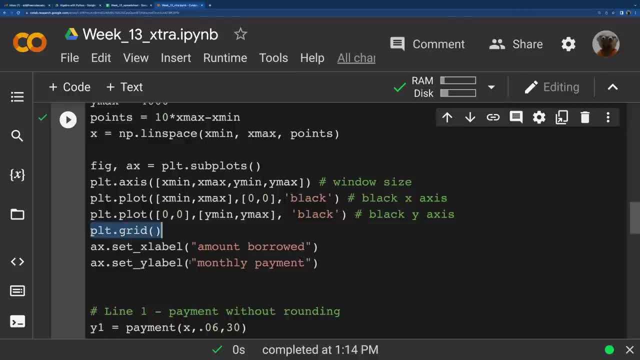 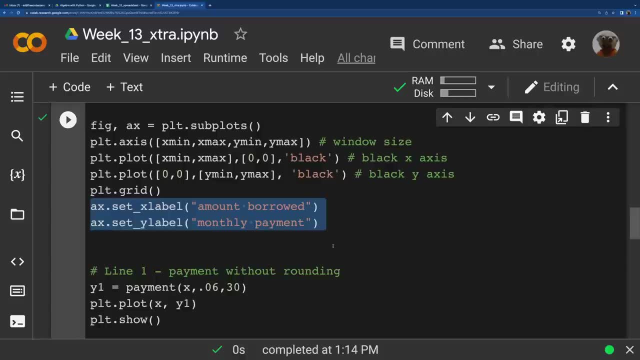 Something that I don't always put in there. pltgrid Just to show the grid lines And XsetXLabel and setYLabel. So the X will be the amount borrowed And we see that that goes from $300,000 to $300,000.. 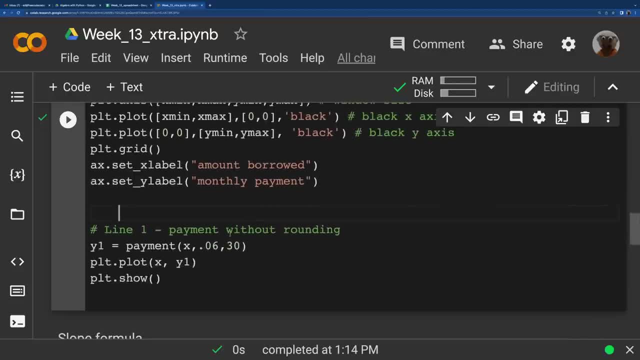 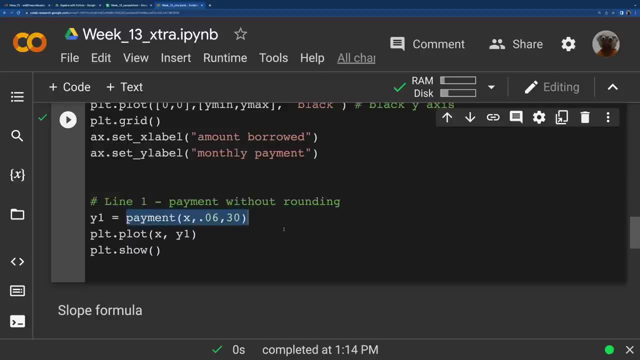 And the Y will be the monthly payment. So now that payment function I defined earlier, I can just use that as my Y value. I only need the X that I'm going to use as a variable here And I'm still going to give it just a consistent rate and time. 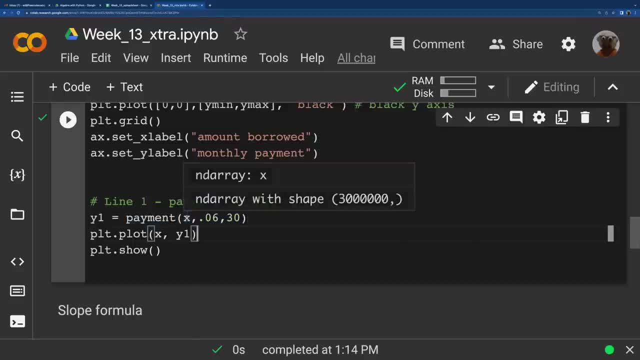 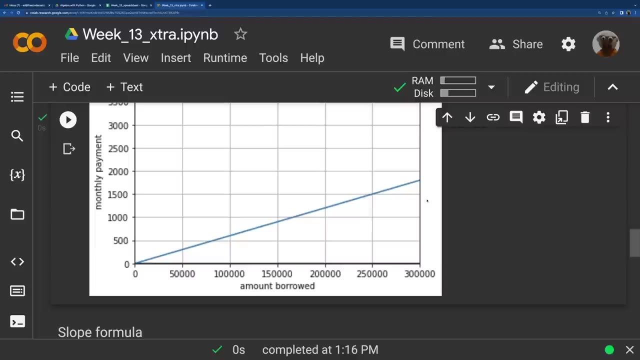 So you know, X is the input. All of these are going to be given the same rate and time. How does the principal affect the monthly payment? And when we run this We can see that the payment change is actually linear, Given that same rate and time. 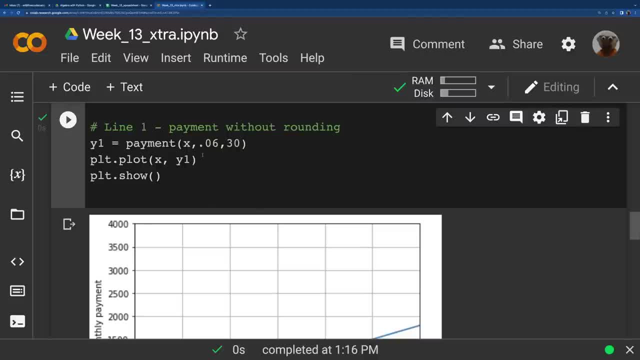 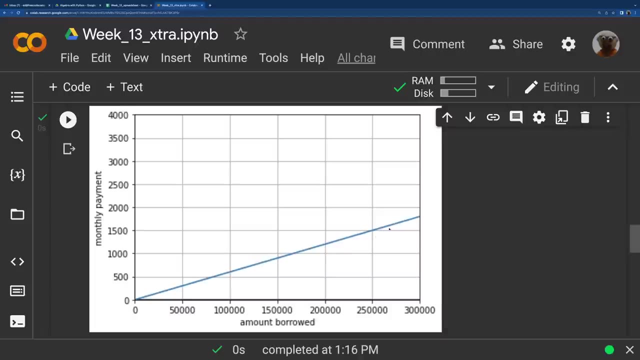 And this would be realistic. Maybe you get pre-approved from the bank, So you would know your interest rate And you would know the time. So just comparing different mortgages, it is linear. How much would it increase? You know how much would the payment increase for increases in the amount borrowed? 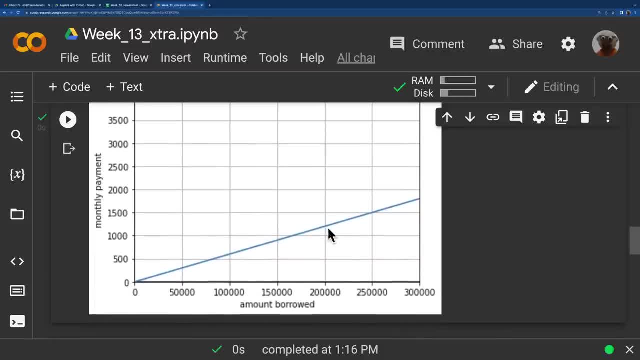 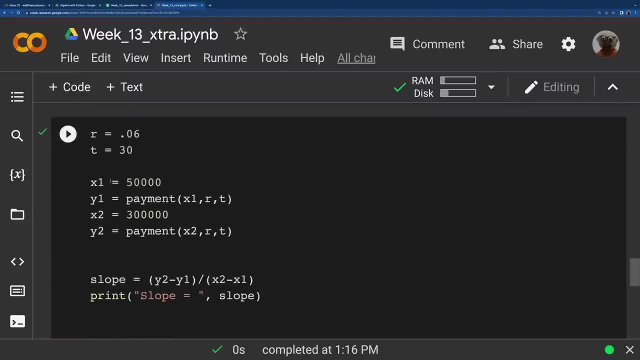 Well, all right, this is a good visual of it, But let's get down to the numbers. So it's linear. I'm just going to do the slope formula And I'm just going to pick two values, You know X1 and then the payment. 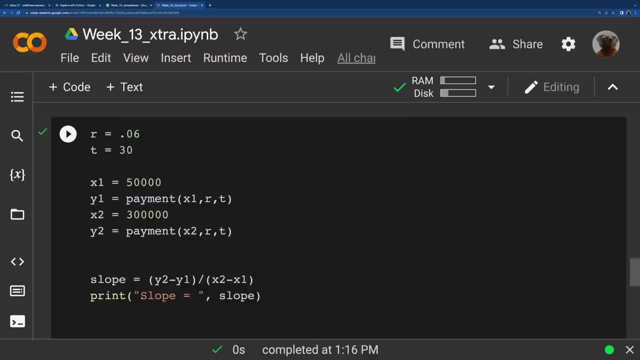 And notice this. I just put rate and time here And I define them up here, Just a different way of doing it. I'm using the same numbers consistently throughout this. I feel like that would be good for the consistent example. And just pick two X values. 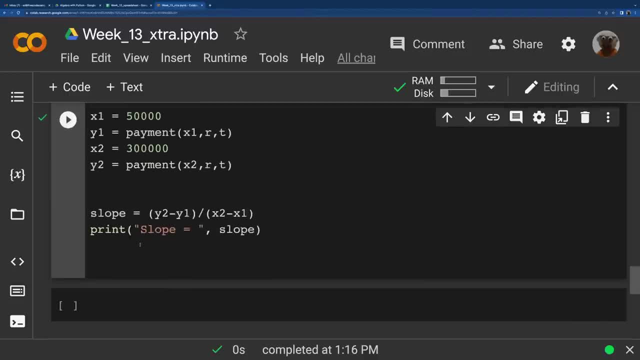 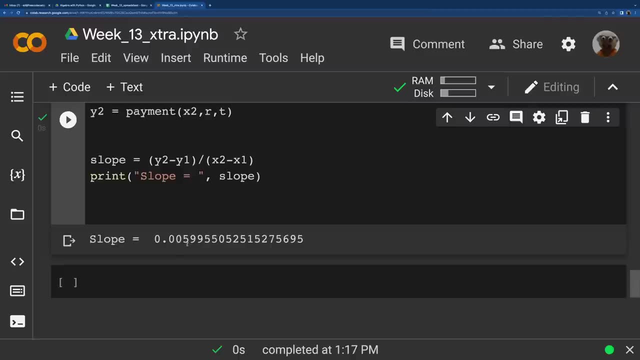 Calculate the payment based on those X values And calculate the slope formula And what we'll find. So, without rounding Now notice this is: You know Dollars and cents, So really it would go up you know $0.06 for every $10 of you know price increase. Or we can, you know, multiply it by $1,000 here And say it would go up $6, you know, because $5.99, I'll round up It would go: Your mortgage rate would go up $6 for every $1,000 extra you borrow. 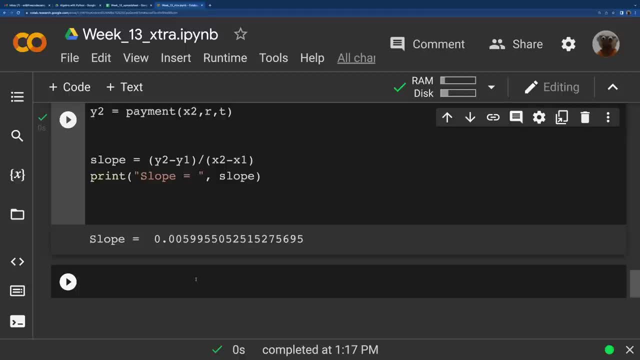 And now you have that in mind. Oh, okay, An extra $1,000.. That's going to be an extra $6 in the monthly payment, And you know you can put things into perspective. Do I like it that much? 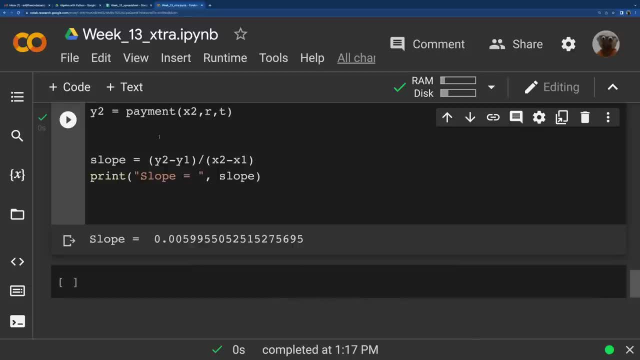 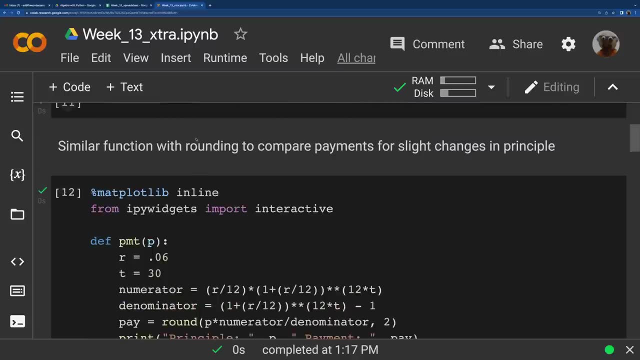 You know, oh, the extra $1,000 is only $6 more. So we see some things we can do with this. We can take these formulas that we've been working with And we can define them as their own functions. 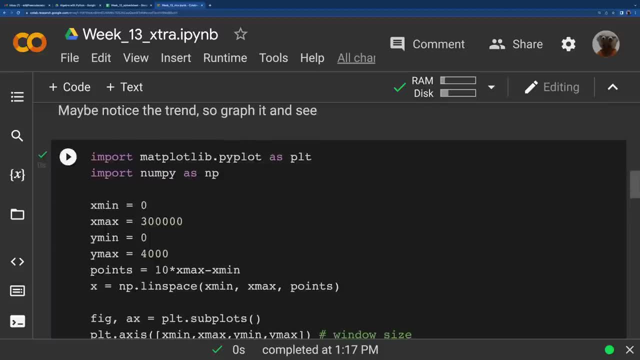 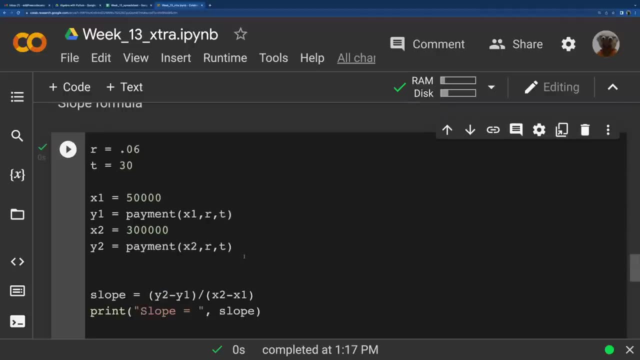 We can use them in sliders, We can graph them And, finding aspects of the graph, we can do other analysis. This is kind of like what we want to be building upon for our data analysis. So this is all good And I want to actually then have like a bonus here beyond the Python. 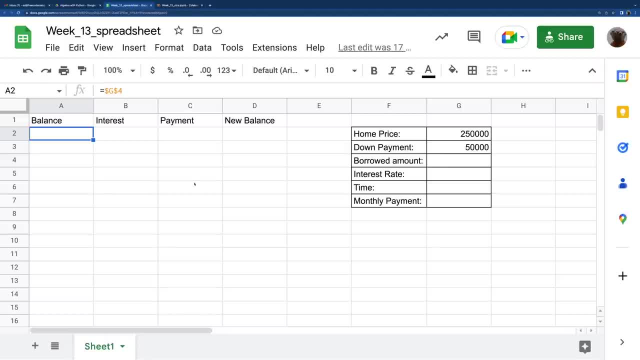 I know this is almost all Python, But I want to get into showing how you can do this in a spreadsheet, Because that will give you, like that, full amortization table, And I want to show you also How to build that, because these are some good spreadsheet skills you'll want. Okay, So notice the balance. here is a formula, but we'll get to that in a second. So, given that, given a home price, I picked this $250,000.. That's somewhere around the median home price in the United States right now. 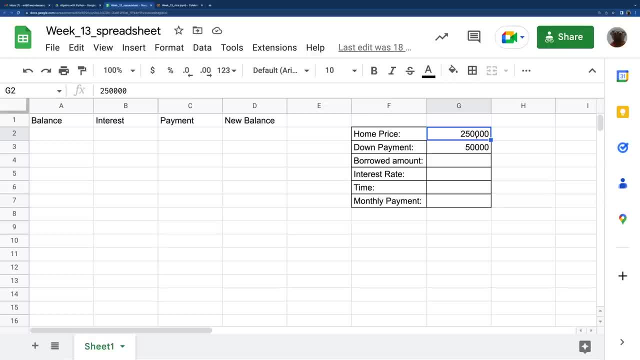 I want it to be some realistic middle of the road number Down payment it's going to be. we want 20%. So notice, if I click on this, This is cell G3. up here is the formula and I just did: 20% times G2, 0.02 times G2.. 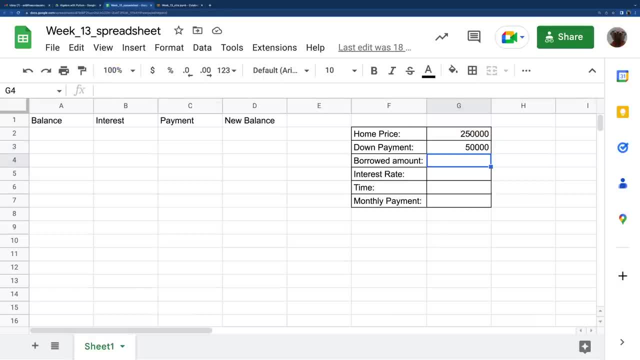 So that way, if I change this and I make G2, you know, 300,000- instead click somewhere else, then it will automatically calculate the down payment. I think I do want to go back to 250,000.. Again, that's. I feel like that's a good middle of the road number. 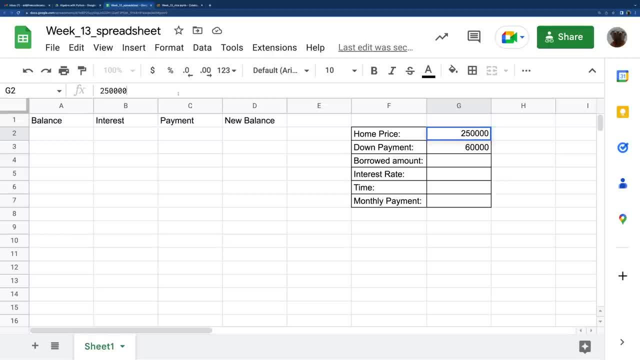 For us to use as our example and click, and it'll adjust again. Now, then the borrowed amount- I would subtract that, So I'm going to double click in this- and equals G2 minus G3.. Actually, that's exactly what I wanted. 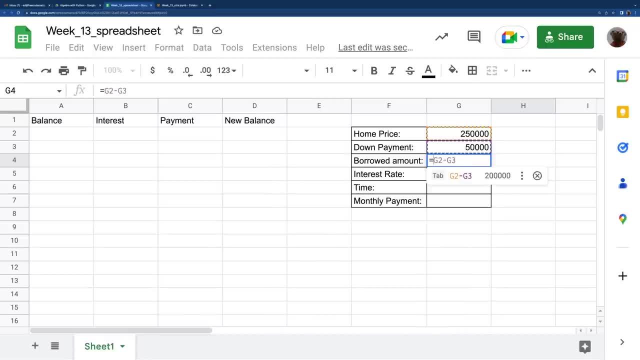 Sometimes, sometimes Google will prompt, you will give you that And notice that I can click on this and you can see the borrowed amount. And then up here this is the formula G2 minus G3, which is the home price minus the down payment. 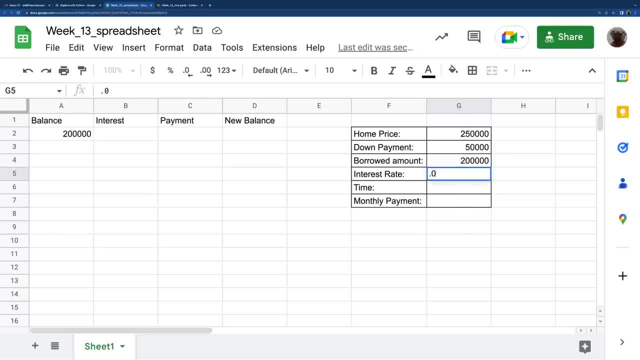 All right. So let's just say the interest rate. you know 0.06 and time: 30 years. Now I'm going to write the word years here. I'm not going to use this number for anything else, But here the interest rate, I will. 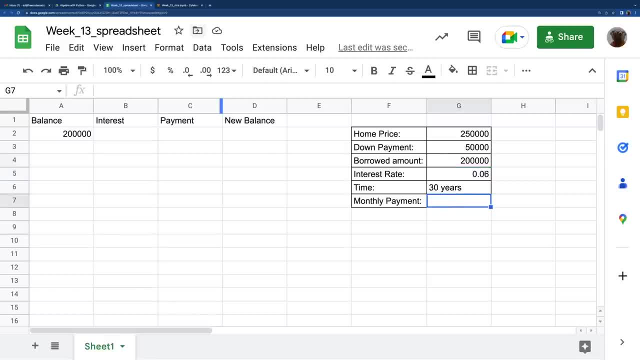 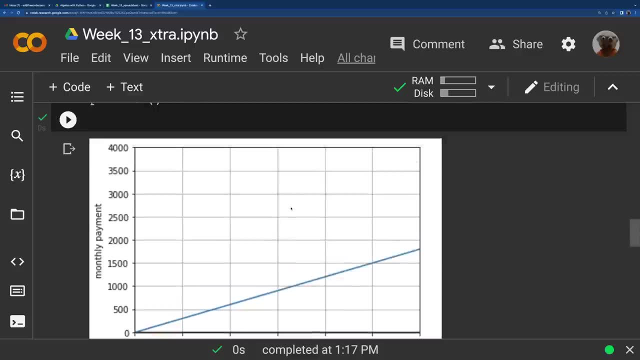 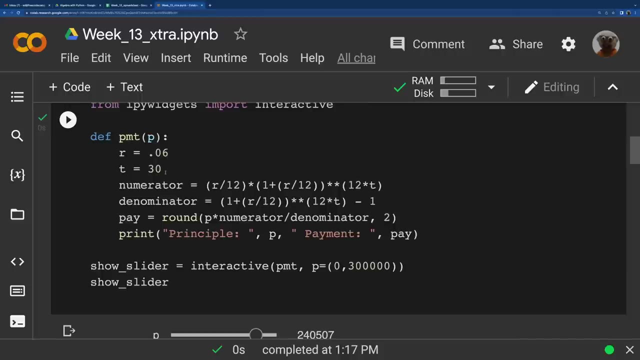 All right, Now monthly payment. We can always then go right back to this and calculate the monthly payment. So we see, here I just had this monthly payment. There you go: 6%, 30 years, And I already have this. 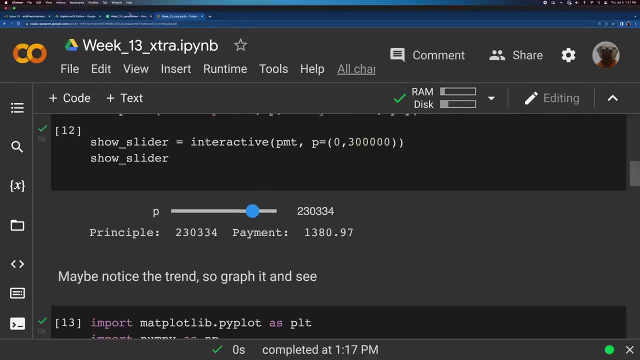 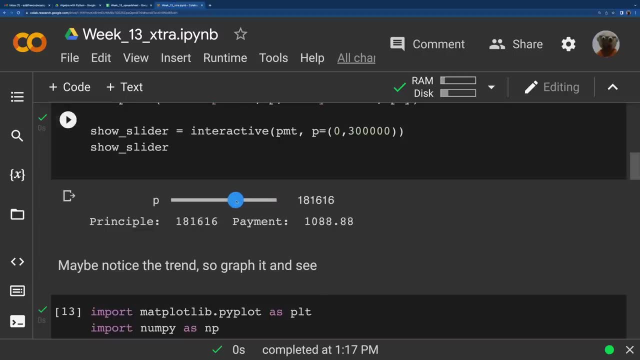 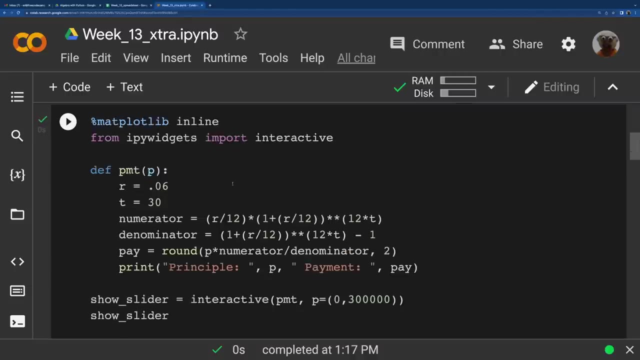 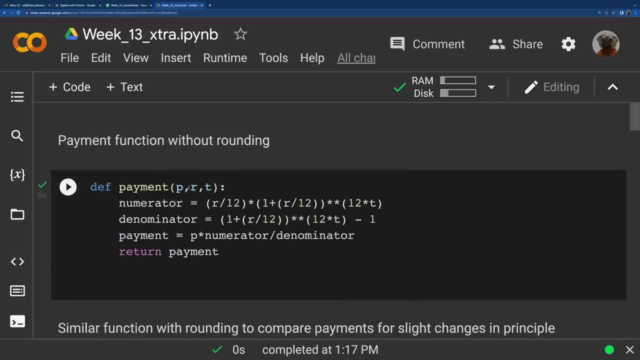 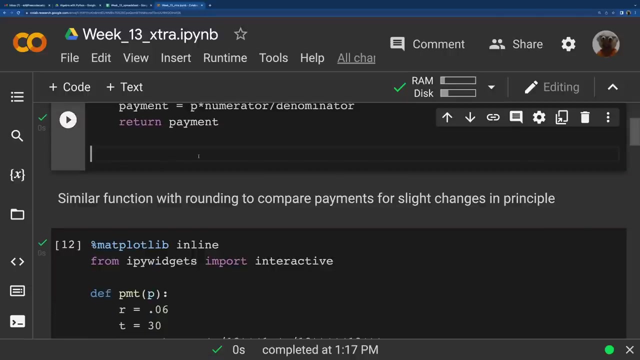 So what if I just made it my borrowed amount, which was 200,000 even, And I can just go to this borrowed amount 200,000.. Now I could actually also just make another, Since I already have that payment. I could actually, right under here, write print payment. 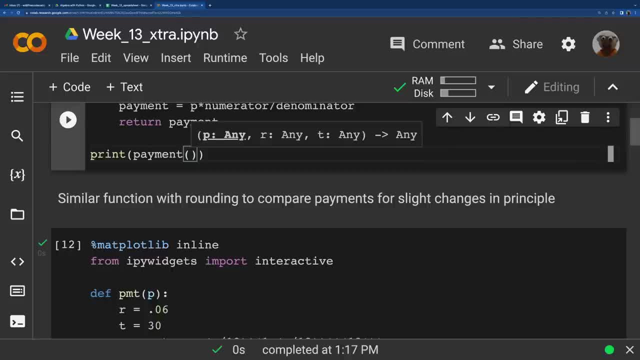 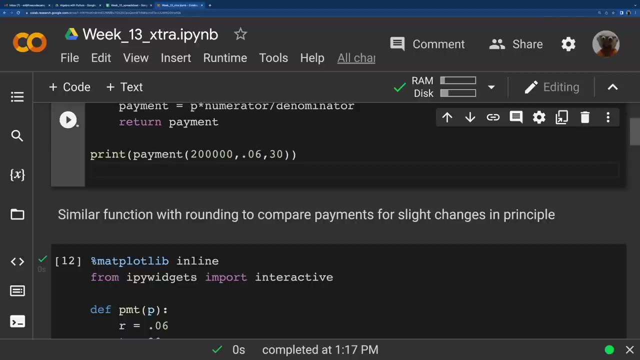 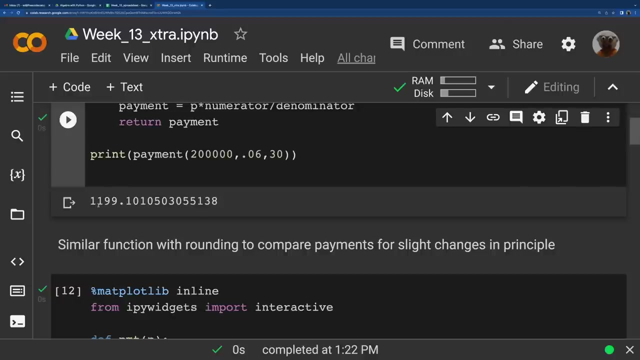 Payment 250, 200, comma 0.06, comma 30. So you see, I could just actually just put this in here and output the monthly payment. All right, There we go. 11.99 and 10 cents. All right, There we go. So monthly payment will be 11.99 and 10 cents. So now notice here: This is just a good reference for all the things we want: Home price, down payment and everything. 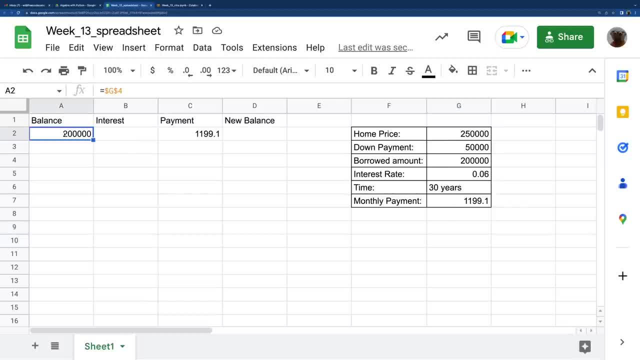 But these notice I already had to just populate over here The monthly payment And, if you'll notice, I have these dollar signs here. That's going to be for some things we're going to do later. I don't need them over here. 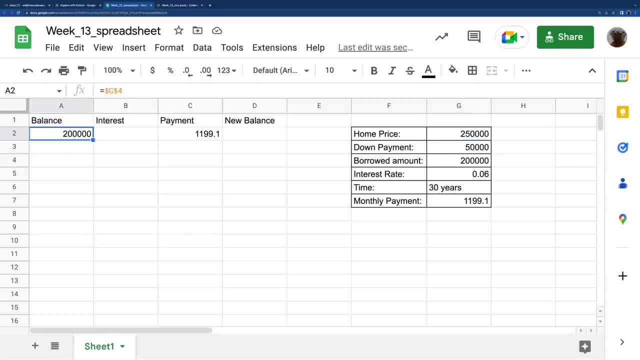 But we're going to do some things later where we're going to drag these formulas down And it's going to adjust according to the row And the dollar sign will keep that the same. So dollar sign G: dollar sign 4.. 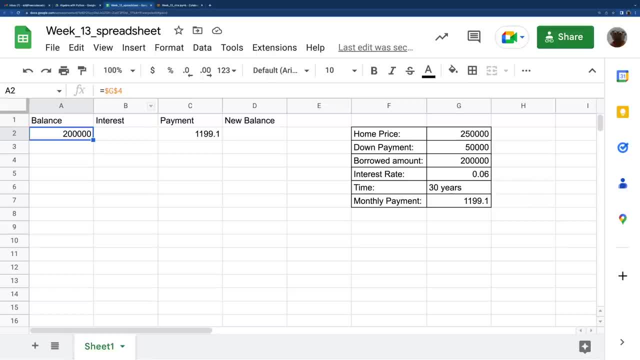 That means if I ever adjust this, that's not going to change. It's going to stay referencing that cell, G4. And same with the payment. That's always going to reference G7. And that's what I want. Now the interest. 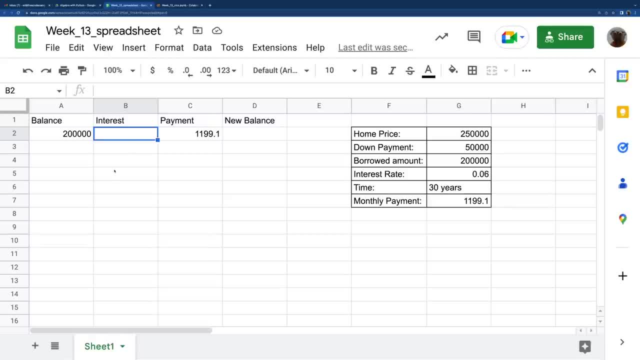 We've been doing all these fancy interest formulas, But actually this is going to be monthly. Each of these rows is going to be a month. So for monthly interest we can just do simple: interest Equals the print, that balance, which is A2.. 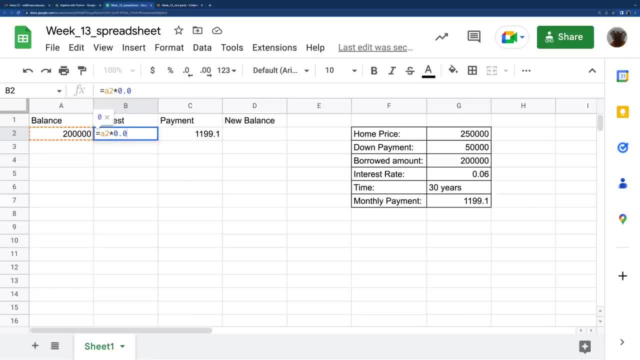 Times the rate which is 0.06. Times the rate which is 0.06. Times the rate which is 0.06. Times the time which is 1 month. So 1 month is 1 twelfth of a year. 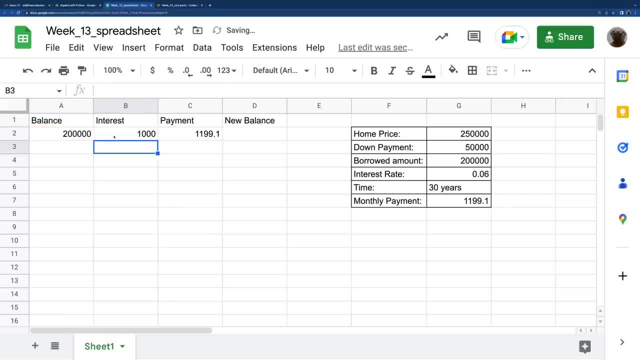 So I'm just going to say divided by 12. And this works out. I mean, that's very nice, But it's not always going to work out evenly. So what I want to do is I want to add another function around here. 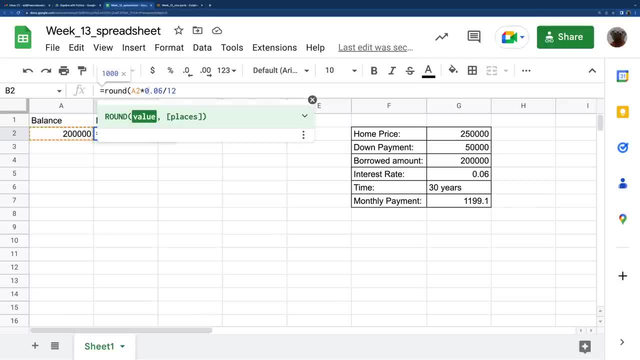 Round- Open parentheses, And I will put you know. so it rounds this And if I don't put anything else, you see, it'll round it to the whole number. But I want to put comma 2. Because that'll round it to two decimal places. 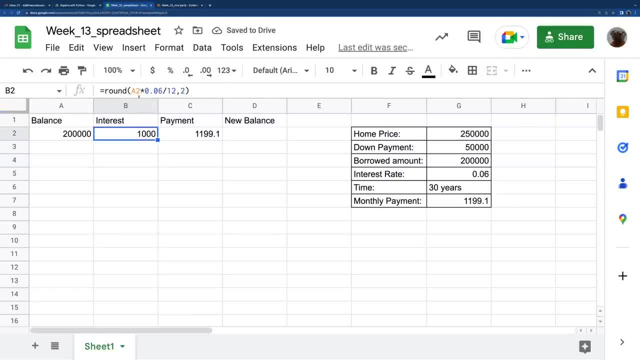 And this is Google Sheets. If you do this in Microsoft Excel, you have to have that comma and then however many decimal places, Even if it's 0. Google, if I eliminate that, it'll just round it to the whole number. 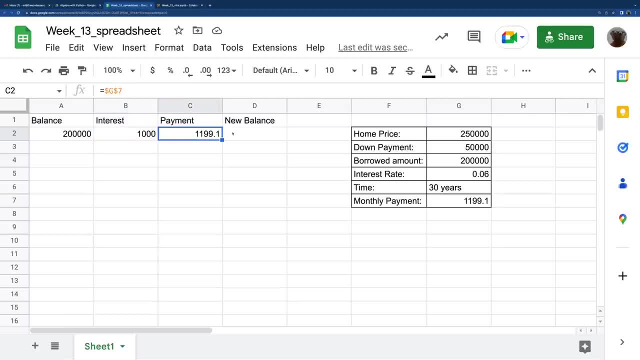 So there we go So round. I have my payment, And then my new balance equals the original balance, which was A2. Plus the interest of the crude, So that's B2. Minus the payment, which is C2.. 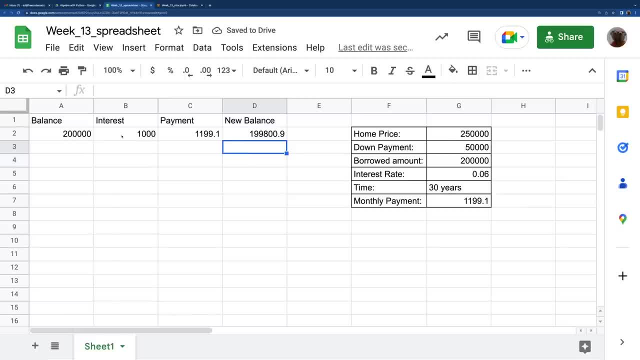 And I want to take this. So we see, you know, earned $1,000 in interest. You know, just Sometimes it's a lot to stop and think about that And all that they paid, you just took a little bit off. 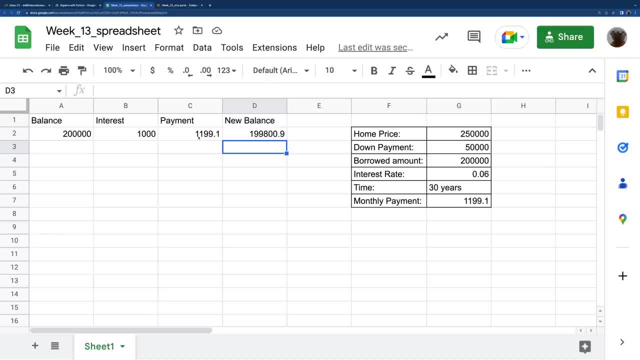 Because that earned $1,000 in interest And then the payment was only $1,199.. So a little bit of that- like $200, went to paying down the original principal. So I want to take this, Because then we have the balance. 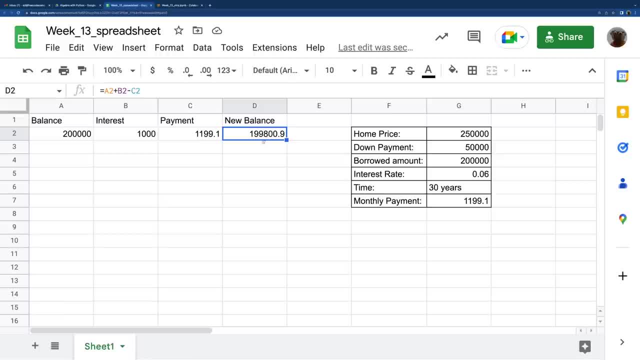 It accrues interest. I make a payment, New balance- And I want to take this and carry it over here. So that was cell D2.. So I'm just going to put equals D2 here And here. now notice if I drag this down. 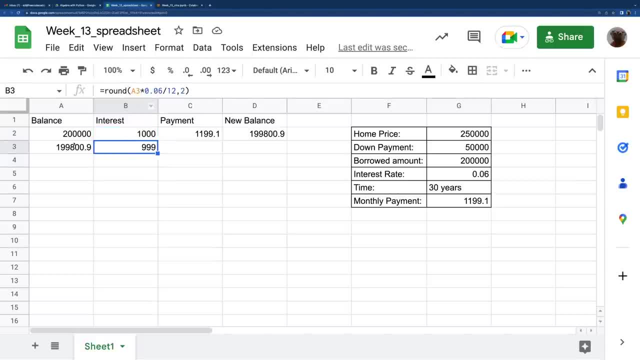 It changed because it's calculating the interest now based on this balance. You see A3 times 0.06 divided by 12.. And then here, when I drag that down, it's going to be the same, Because I put the dollar sign in there. 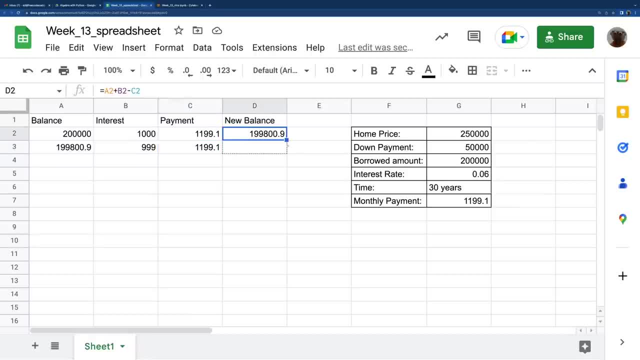 It won't adjust anything. And here I will drag this down one And we see again doing that. it adjusts it for this row. Now, everything here was based on row 2.. Everything here is based on row 3.. 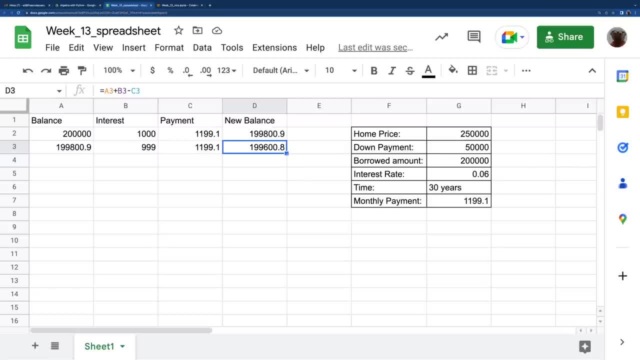 And we got that. by mousing over the bottom right-hand corner You get a little tiny plus sign And this is magnified. But you know you'll see that thin plus sign And you click and drag that. But we're going to do that for the entire row. 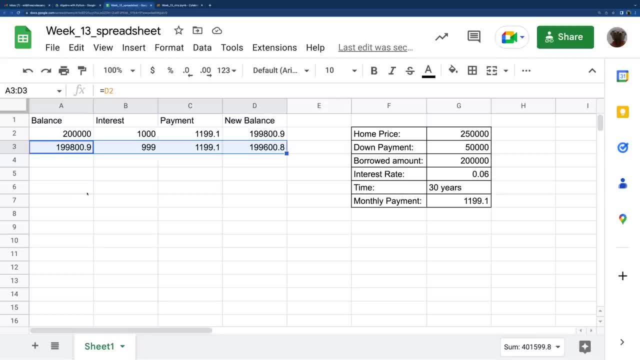 So I'm going to hold down shift and the arrow key to highlight the entire row And I'm going to mouse over that. I get that thin plus sign And I'm going to click and drag And this is how we make our amortization table. 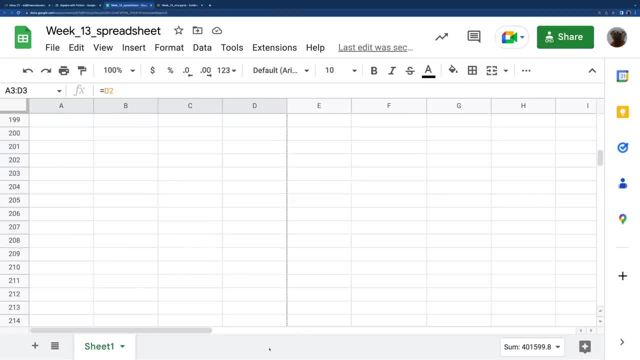 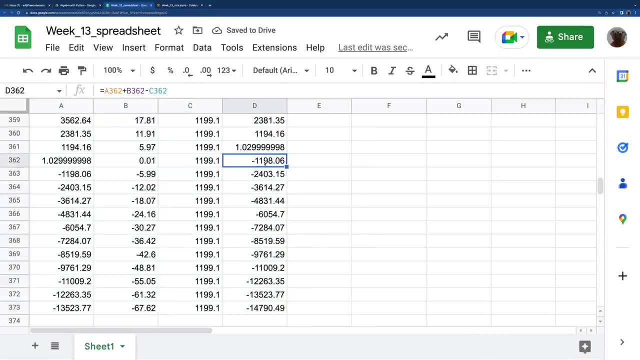 Now notice my mouse is down below the bottom of this- Because for 30 years, that's 360 months. So somewhere around there Around, there is where I'll stop, And these are all negatives, So I'm going to take this. 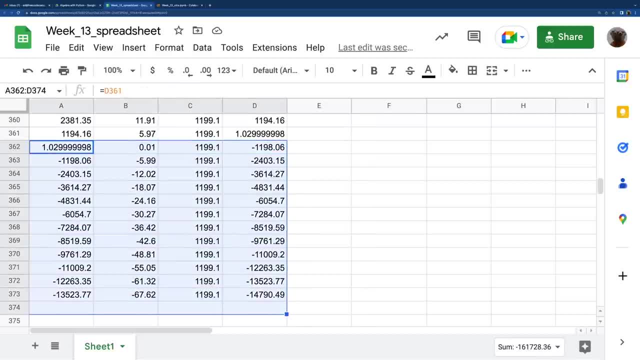 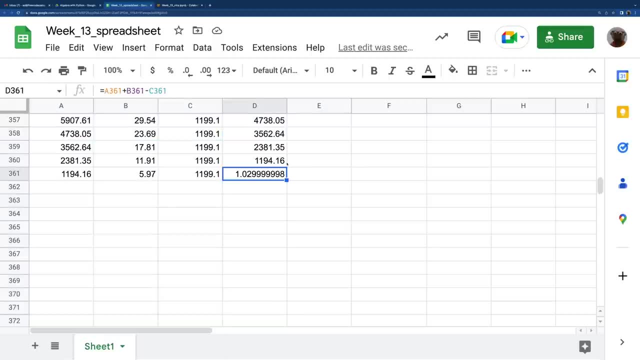 Highlight all these negative numbers And then just delete them. So now, here this is. you know, after this, the balance is a dollar, So we can just make this $1,199 plus that additional $1.13.. 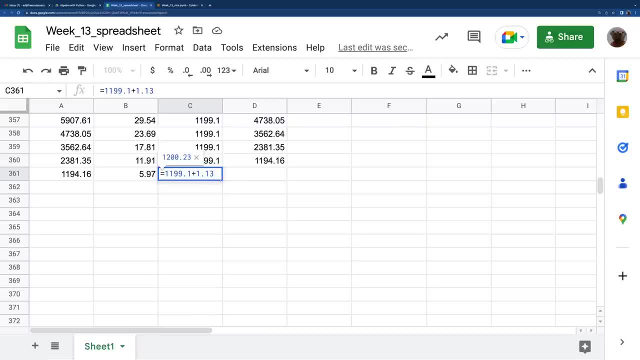 And I'm not going to take it to multiple decimals like that, And that should be: Yes, Ten cents Negative, ten cents dollar three. And that should be enough to make that. We're just going to call it That many zeros. we're going to call it zero. 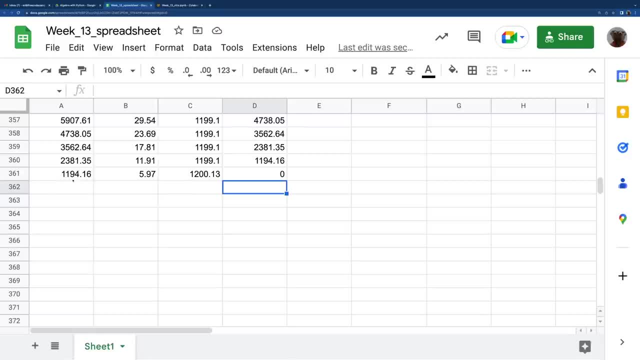 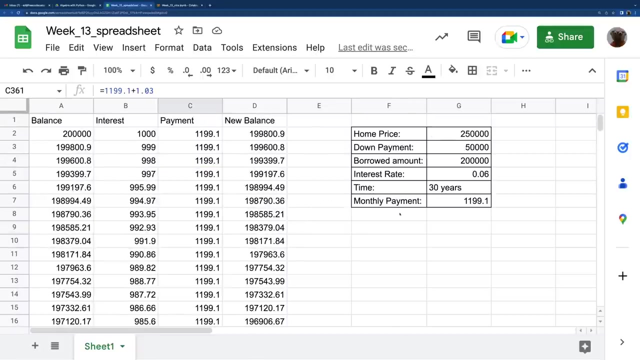 And what we have. the row number is always one more because we had the first row as headings. So, given that mortgage payment, it works out exactly 30 years, exactly 360 months. You have a balance of zero. So we're going to take this. 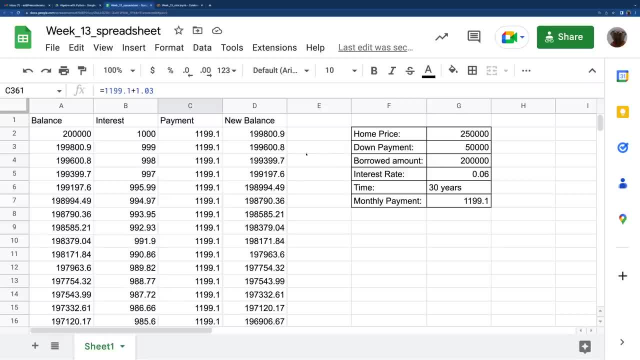 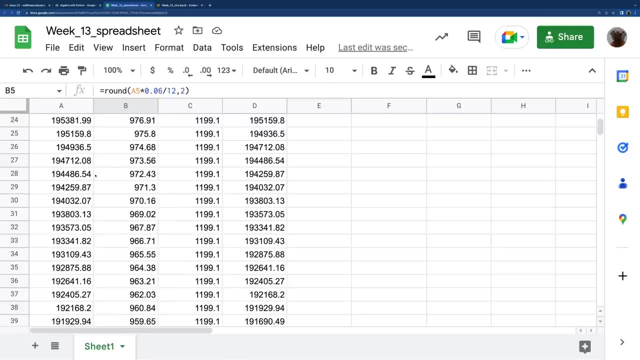 And we see this is the amortization table And you know you can look through it and scroll through it and see how the payment stays the same, But what happens is the amount of interest keeps going down gradually Because for such a large amount of money for such a long period of time every month, the fact that you're paying interest on just that little bit less, that really makes a difference. 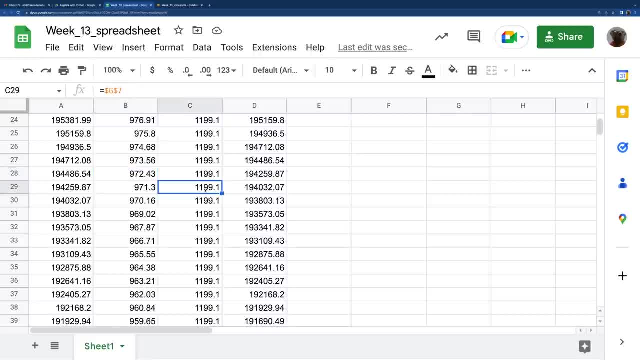 And then that means that you know that same payment, a little bit less interest, a little bit more of it goes to the principal. So you know you're making some progress paying this off, But it takes a while until See, look at this. I mean that's almost $1,200.. So we have to go into, you know, 225 months. You know we're coming up on 20 years until you know half of your payment goes down. 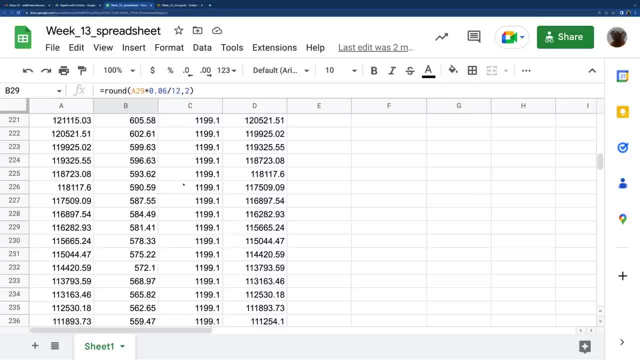 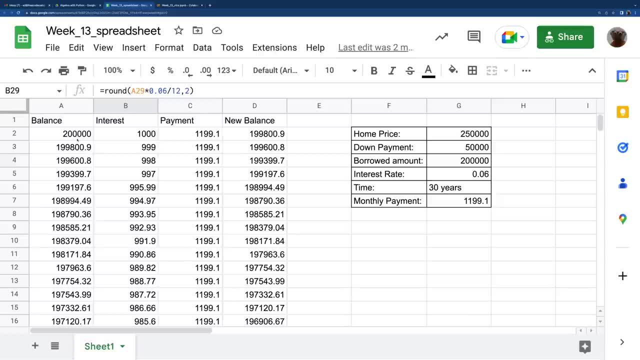 Half of your payment goes to interest, Or less than half of your payment goes to interest. So it's just good, interesting to see that whole table And then this balance here at any given month. that's the payoff amount, You know, supposing you come into some money and you say, oh, I just want to pay off the rest of it. 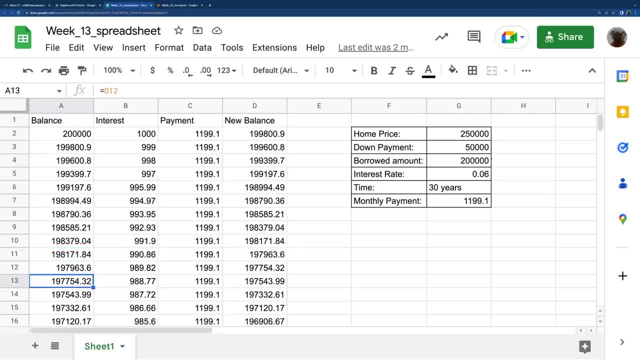 You know, that's the balance, That's your payoff amount, And we have all this Now, besides showing you the spreadsheet and how you can set this up And how we can, you know, grab values from other cells, And how we can add formulas. 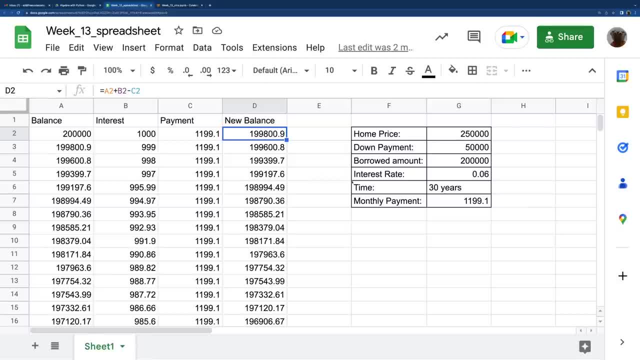 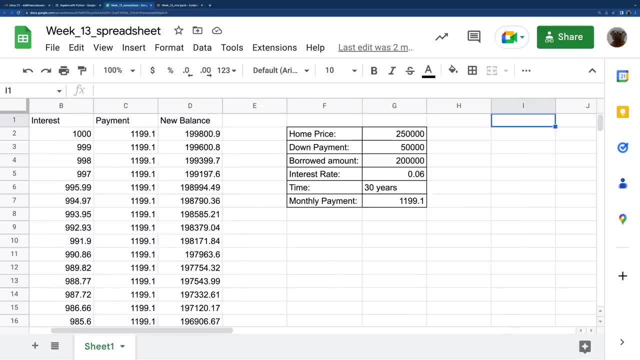 And how we can drag all this down. That's great Amortization. And you know mortgage Mort, You know it does sound like death because you know it is the same word, mort. So let's do something more positive with a very similar type of formula. 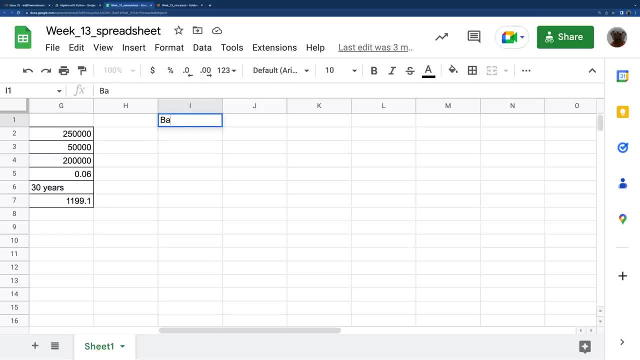 So suppose I set up the same thing: Balance, Interest- I'll capitalize it- And payment, But I'm going to say contribution And then new balance. So let's look at this in a more positive way, Supposing this was this amount that you owed that you're paying off. 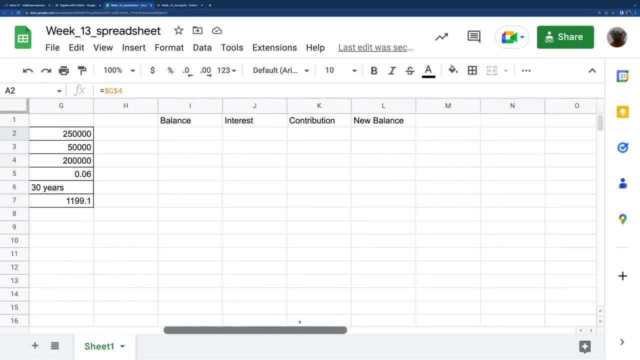 But let's talk about a retirement account that you're adding to, So I don't know. Let's start by some like round number like $5,000.. And a lot of retirement accounts, you know people managing it could, you know, get like 8% interest. 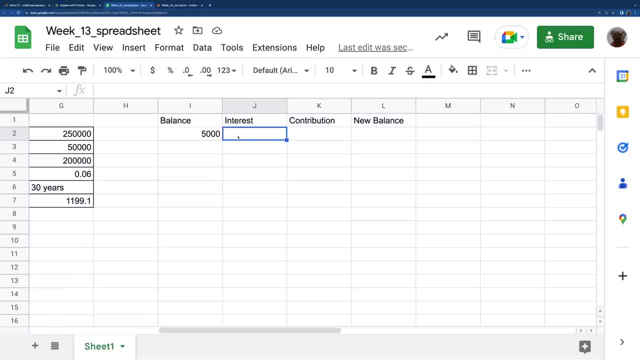 That's pretty reasonable to think of. So we have equal. So we have equal. So this is column I2 times 0.08.. 8% interest, And then for one month. So then you know one twelfth of the year. 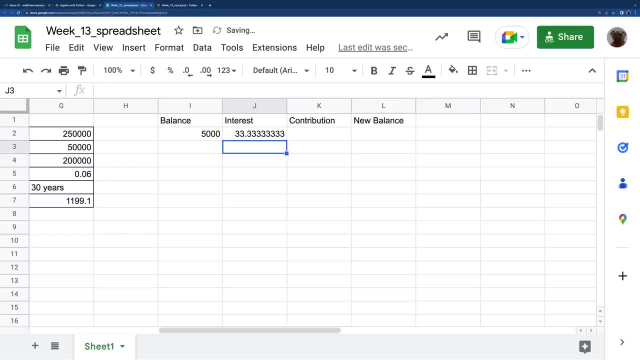 So divided by 12. There we go, And maybe you know we could do this with or without rounding. I'll round it. That might work out. It'll just look nicer Round. And I'll round it to two decimal places again. 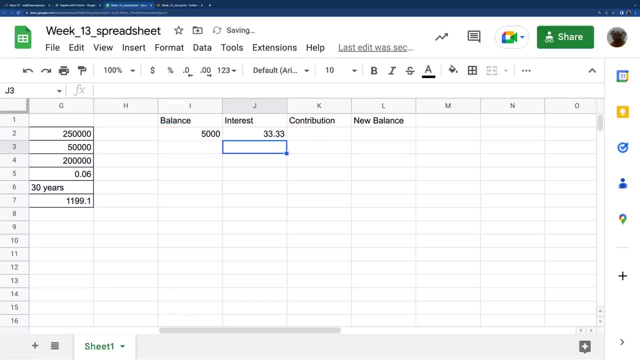 Dollars and cents. Okay, Now monthly contribution. So, who knows, Like you know, you can contribute a few hundred dollars. Let's start with something like this: Like. let's start with like 200.. And we're going to change that later. 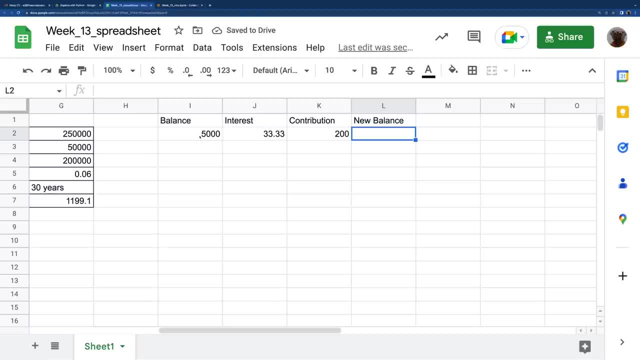 So with balance it gains some interest and you contribute. So it's all plus equals I2 plus J2 plus K2.. And then we're going to carry that around, So that's L2 equals L2. And we're going to do the same thing. 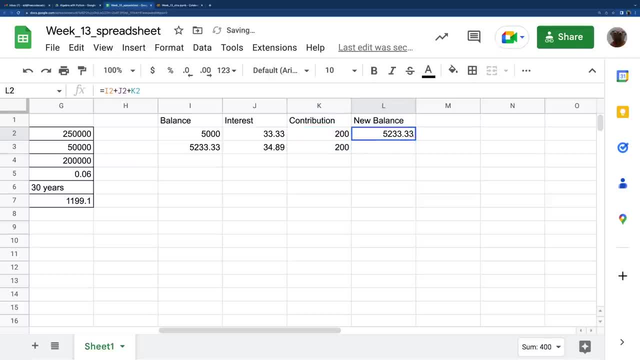 Drag this down one, Drag this down one, Drag this down one, And what we have is, you know, given that, you know rate of interest, given the contribution, you could always add more different times, But I want to show you this for about the same amount of time. 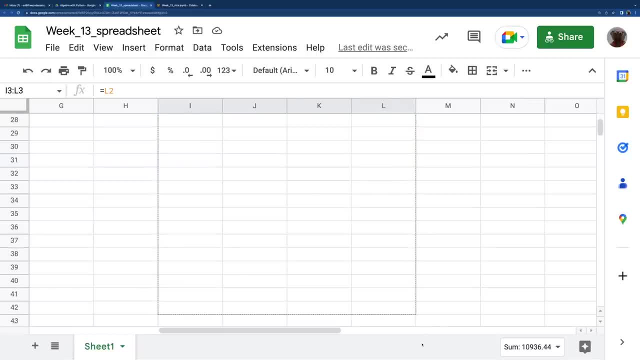 So if we drag this down Now, this being a retirement account, a lot of times people will start this earlier, So we don't really even have to stop at 360.. Let's stop at like 400.. Nice even number there. 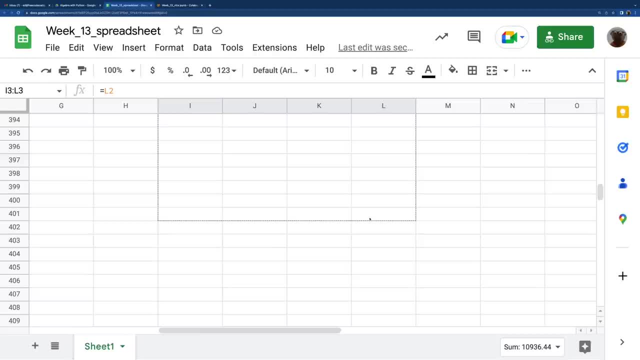 There we go, 401, because the first row is. So what we have is this. At that point, then you know, this amount that you have is $469,000.. And the interest every month is $3,000.. 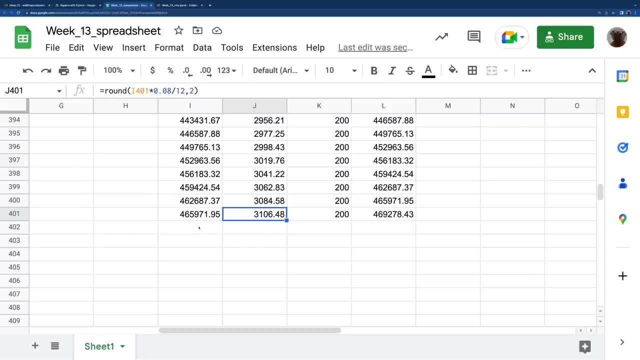 So you could easily like take that interest and then you're back to $465,000.. You know, take that $3,106 out every month And live on that And then you're back down to this. So you know it goes from this and then back to this. 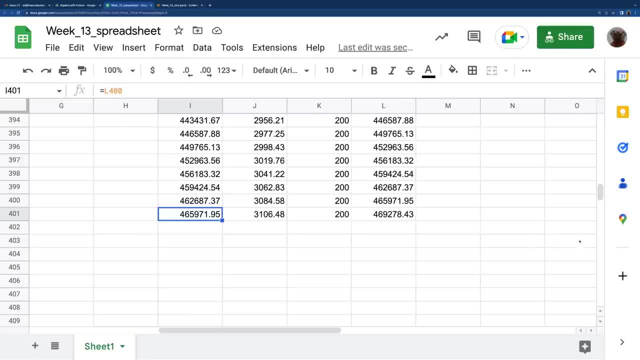 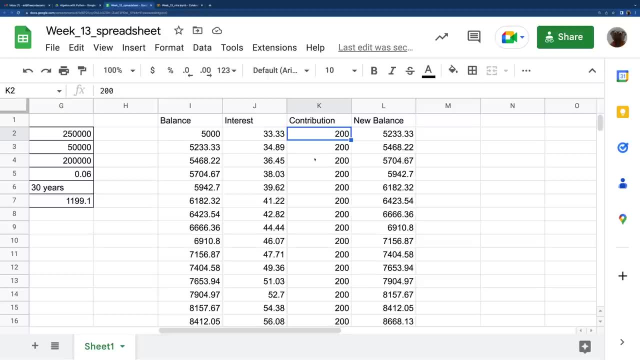 Take that out And then you're back to this. That's one way to do it I just want to show you. So let's get even more optimistic here And say: then we contribute something like you know, $400 a month. 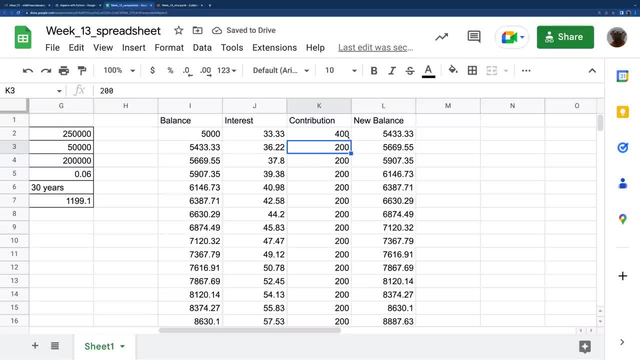 We're going to drag that down in a little bit. And this one, Let's say, you know .085.. I don't know A little bit more optimistic on the. There we go, Drag that down a little bit, And so now that second row again is correct. 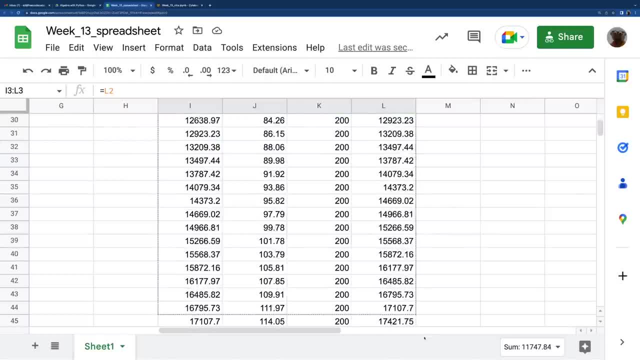 And we'll drag this down. And the other thing I'm going to do is take this a little bit longer, Maybe even like 450 months or something like that. 40 years would be 480 months, So we can take this even further. 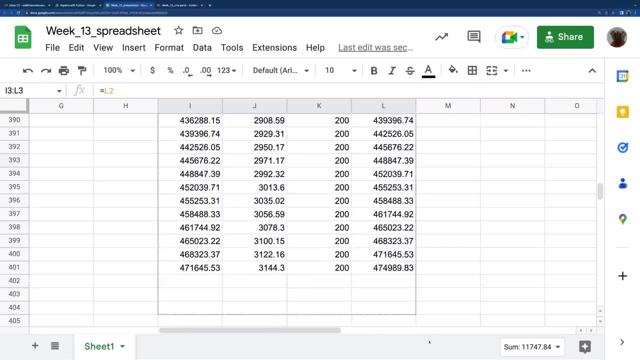 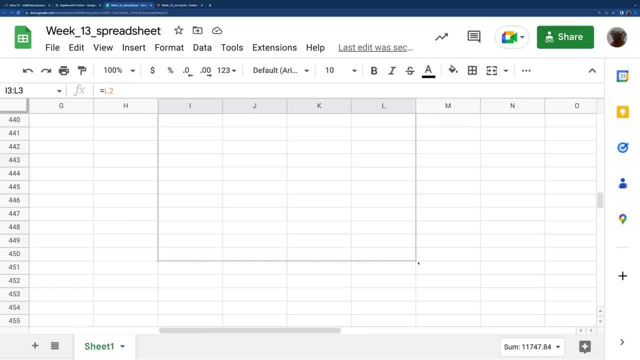 And you'll see that just you know some of these, you know you get some nice possibilities here, All right, And because look at this final number here: So yes, that one is $1 million. So you know, that's what we're talking about here. 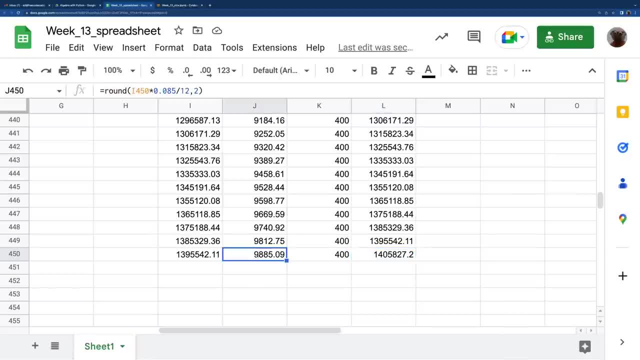 You know $1 million And the monthly interest is $9,885.. So this is something you know. again, I want to, you know, take this same math and turn it around and make it positive, Something that you could be contributing to. 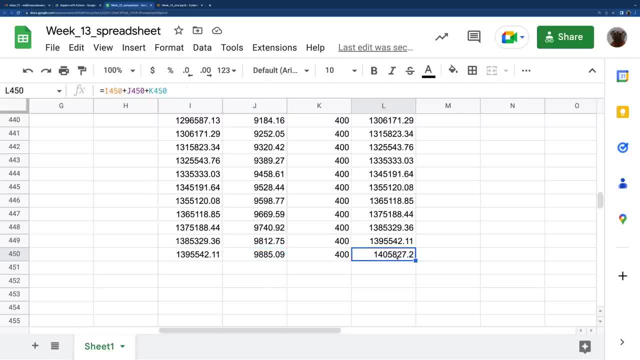 And then at this point you have this money. you know, in this investment You can take this out every month or less and you know not have to worry about it ever running out. Take that out And then you're still left with this. 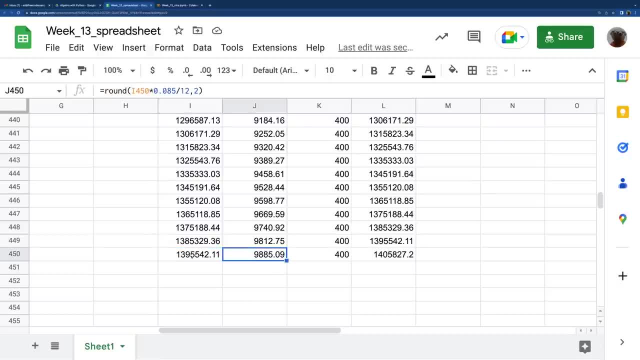 You know more than a million Boom. Take that out. Live off the interest And you still have this every month. Take that out. You still have this to generate interest the next month, And these are some of the things that you can look at that you know from the other side of it. 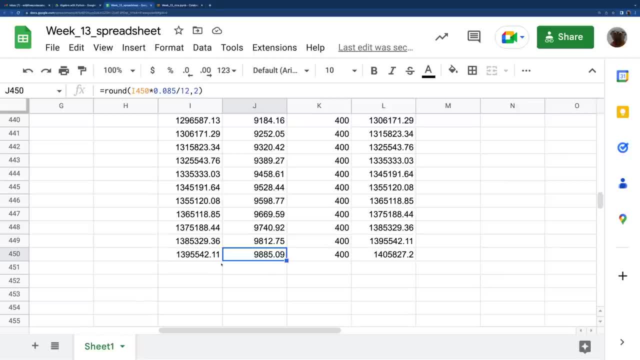 You know you owe all this money to pay off this. You pay off this mortgage, But then you own this house And on the same time you're contributing And you know here. then you have money that you can live off of. 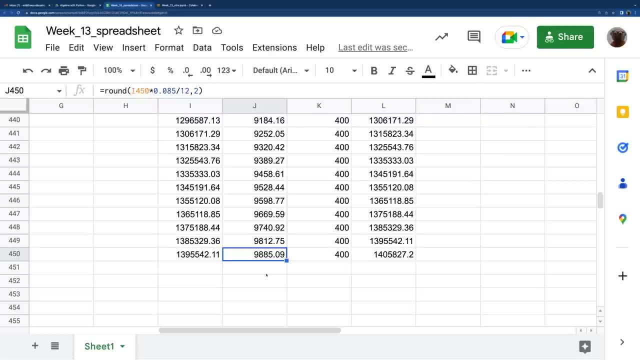 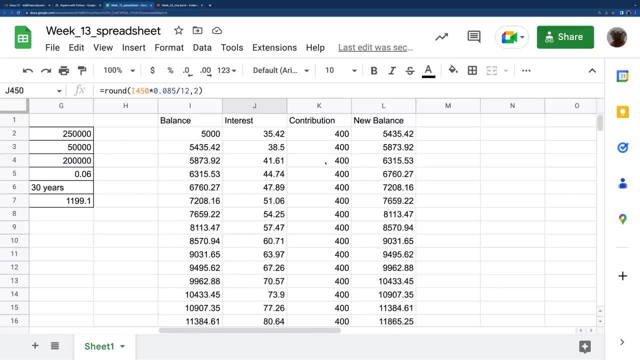 And you know these are the types of things we want to do with our math skills. Look at how we can manage money to you know later on in life than have this. you know property that has equity And you know has value. 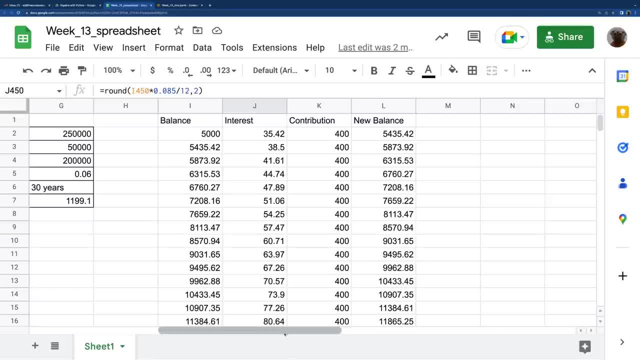 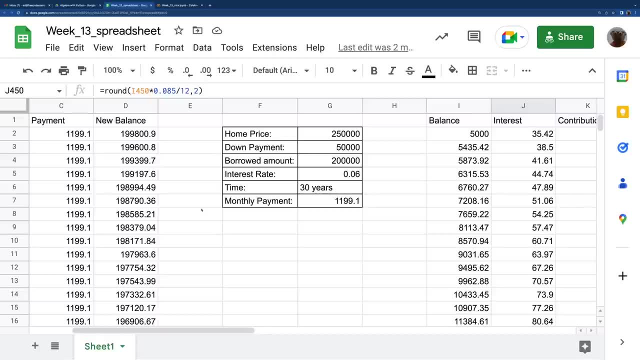 And something else in the bank that you can live off of. And there we go, You know, putting the math skills to use and seeing how you can make this work for you. Seeing the trends that you know, it seems like now you might be working hard and owing a lot and not having that much. 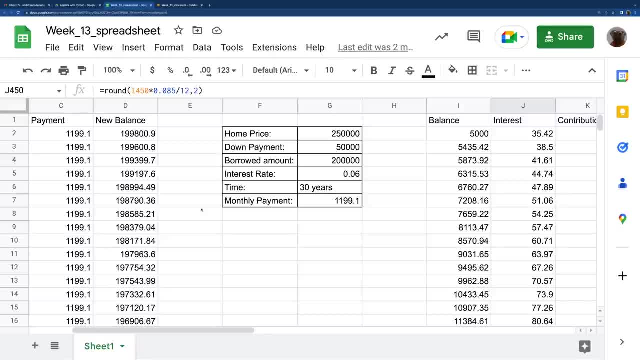 But you know, over time, like many years, you build things And then you have things: oh, I have this that I can now. you know that I've built over decades and can live off of it, So that's really good. 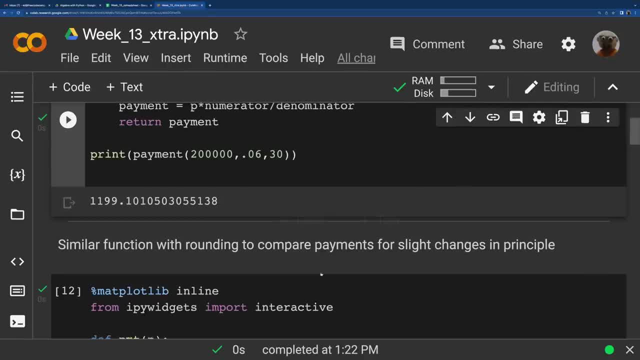 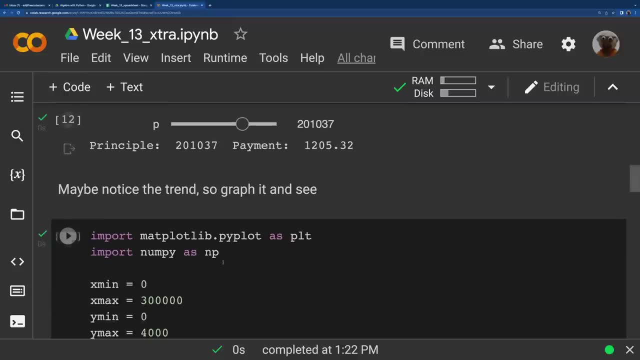 And you know we were doing some of this with the other Python, you know, generating just some of the values. But you see, like these, you know these are some of the ways you can make this work for you. And you know, look at the trends. 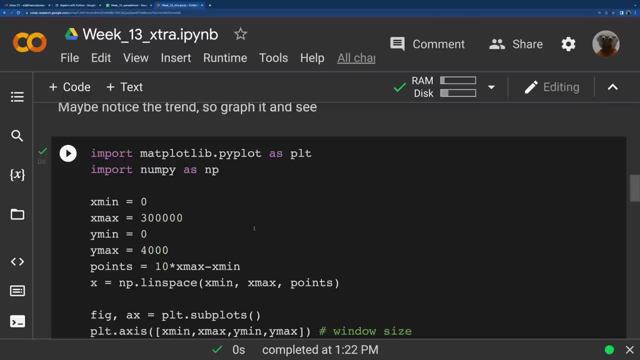 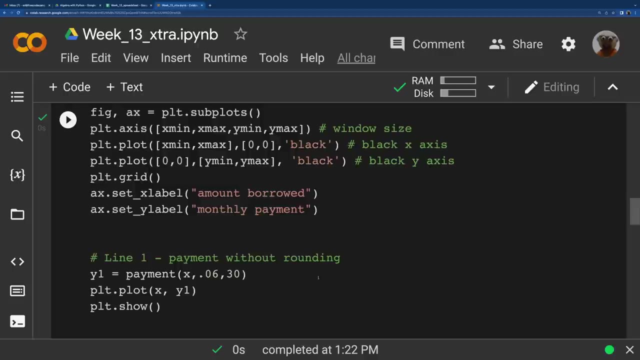 And hopefully this helps you make some decisions about investments. you know whether it be real estate or borrowing money or other retirement investments. All right, So that was just, you know, some bonus, And There we go, We're in the home stretch. 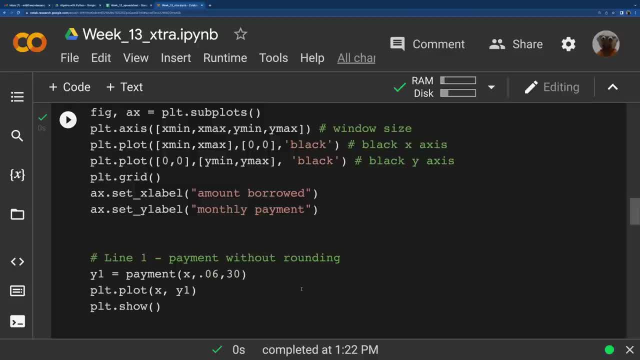 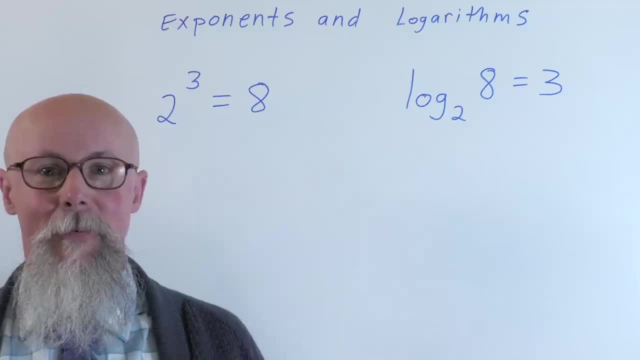 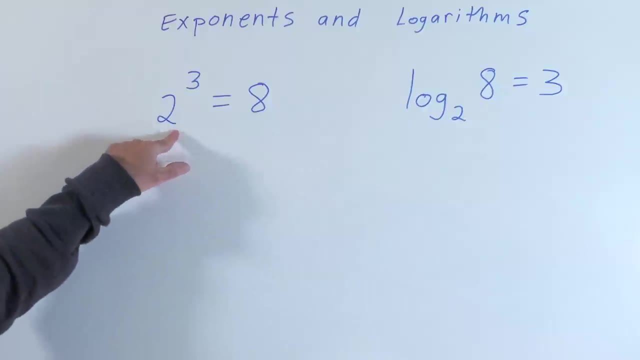 Hopefully you're really seeing this all come together. you know skills that you're building. So let's talk about exponents and logarithms. So the exponential form is this: two to the exponent, three, two to the third power equals eight. So we know how to do that. 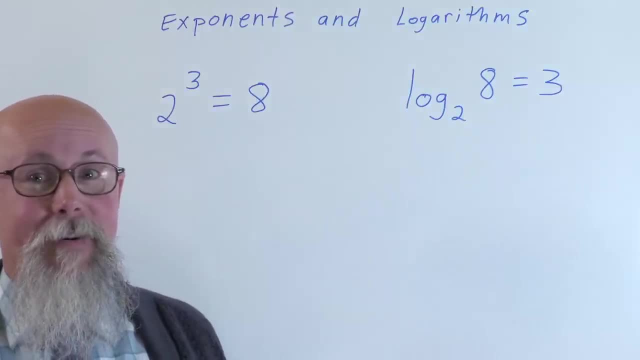 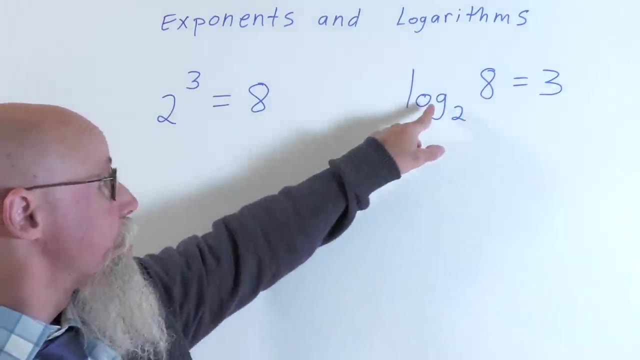 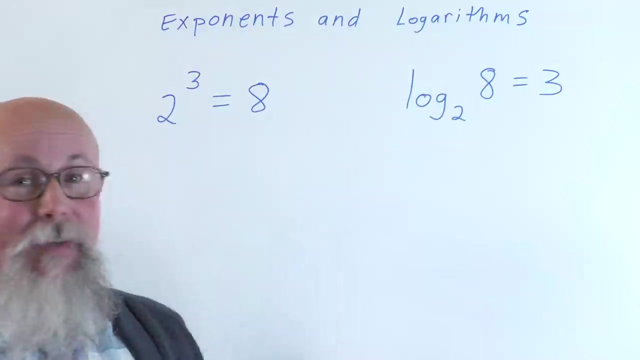 We've been doing this so far in algebra. Then logarithm is the same information rearranged, So this same information, the log base. two of eight equals three, So the logarithm is always: what's the exponent. That's what we want to know. 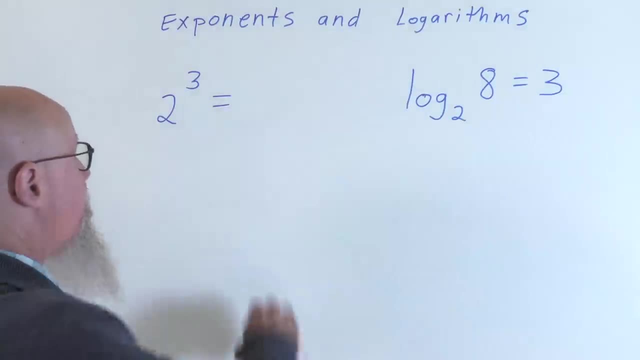 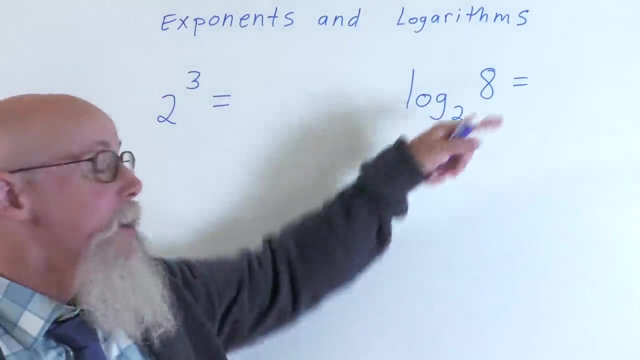 And in what we've been doing so far and in most calculators you know two to the third, No problem, I know how to put that into the calculator in Python. I don't even have to import anything. But if I know the base and I know what I often call the result, if I know the base, I know the result. 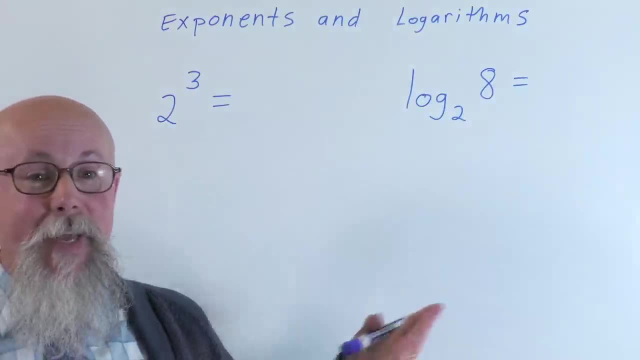 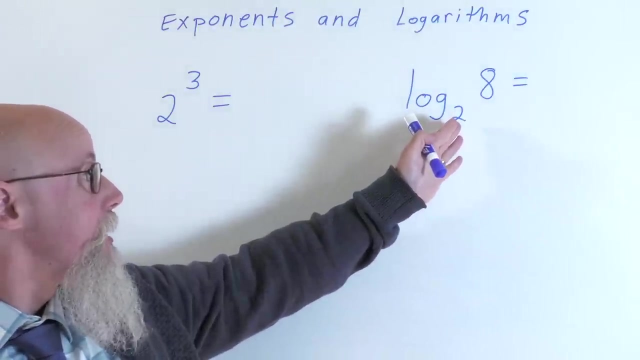 But the exponent is what I don't know. Then that sometimes becomes a problem, especially when it doesn't work out nicely like this works out. But supposing you know it wasn't a eight, you know a nice, nice exponent like three. 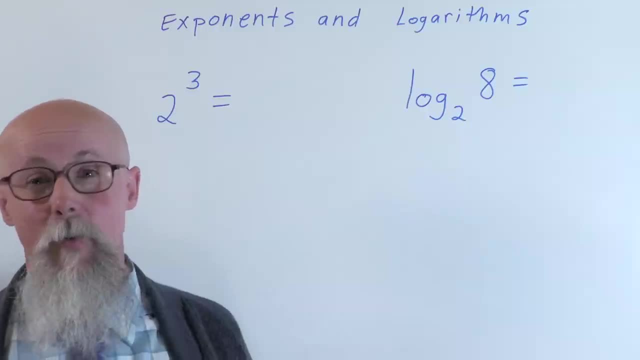 Supposing you know two to the third, Supposing you know two to what exponent gets me nine or ten. It's going to be some weird decimal, But how do I, how do I get that? And so you know, we have to appreciate that. you know, John Napier, you know, spent like about 400 years ago, spent like 20 years of his life figuring this out and making tables. 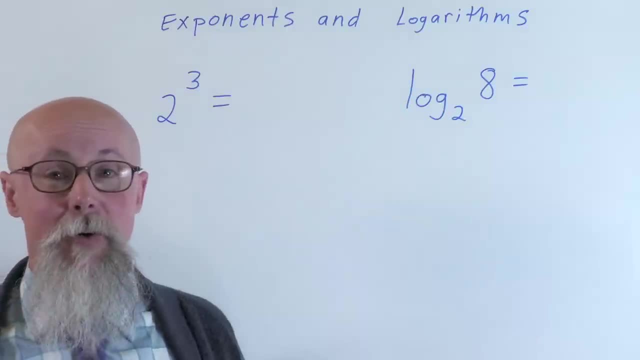 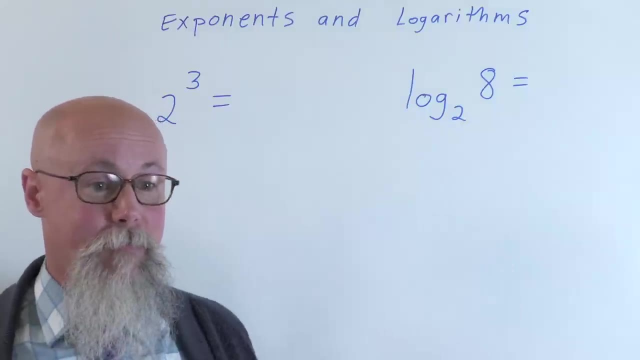 And now we have this at the touch of a button on the calculator And we're going to look at also how to write the code for this. Now, with logarithms, we do have to import something, But you know We'll import a library, you know, much quicker than spending 20 years of your life figuring this out. 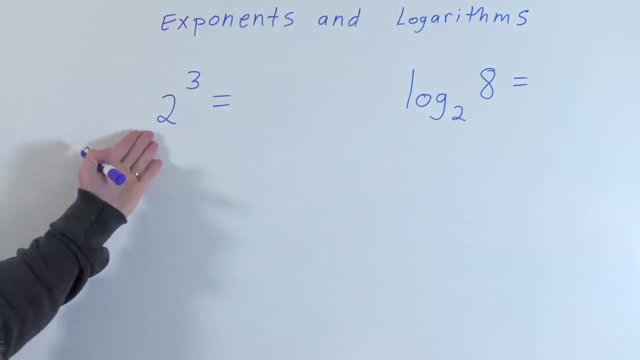 So if we have, you know, two to the third, you know the base is always going to be whatever you know, the same thing with an exponent, what I call the base. So if I have, you know log base two of eight, you know it's what's the exponent. 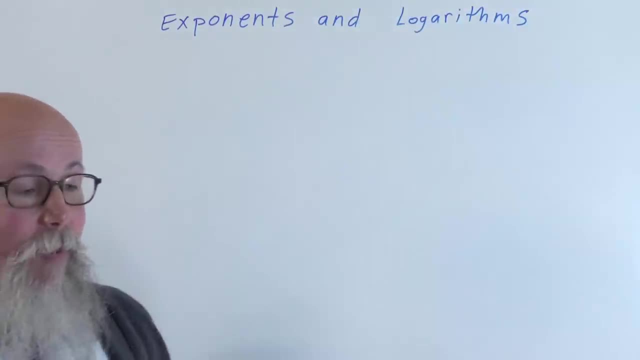 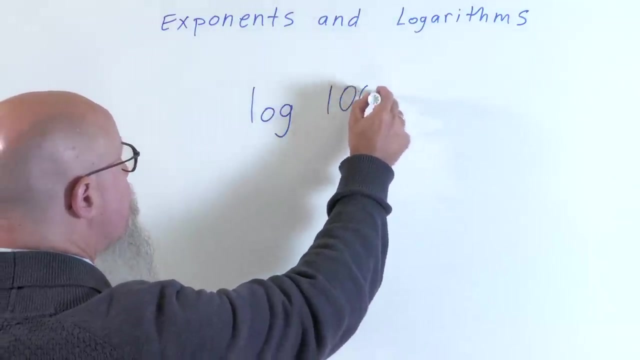 Now what's interesting is our, in our calculators, We you know, you can do logarithms, You can do log. You'll see a log button. Now, if I have the log, if I just say the log of 100 and supposing I don't see any number there, 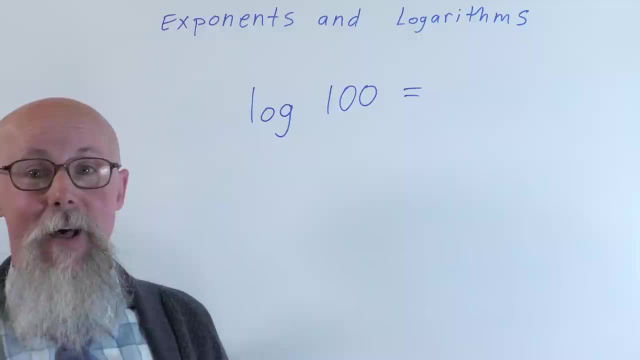 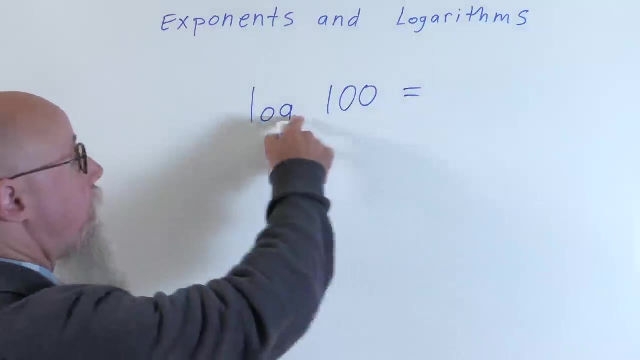 If I don't see a number, then it's understood base 10.. And we call that the common log because our number system is base 10.. So if it's 10, I don't have to write that, And so the log of 100 is two. 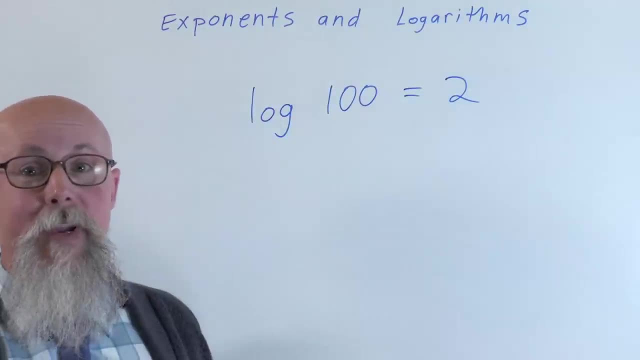 Because 10 to the second power is 100. And we're going to use this a lot of times for working with scientific notation and maybe even converting decimals. So you know that's where a lot of times I'm going to use the common log. 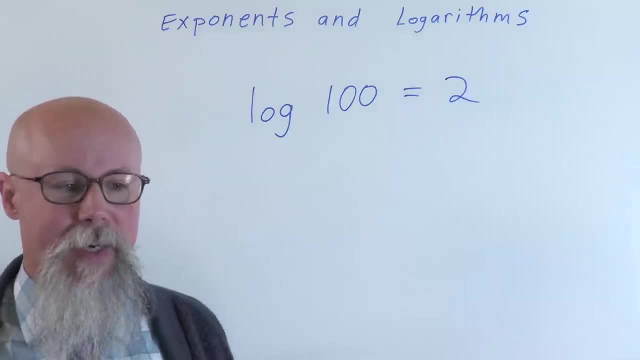 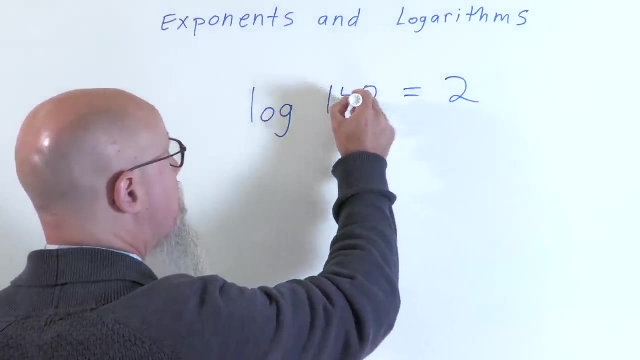 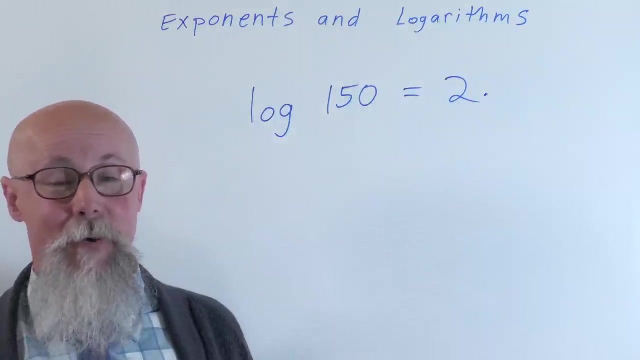 And then I might- even, if I'm doing things like scientific notation, I might even do the floor function, because if you know what's the log, you know like 150.. It's going to be two point something. But then for converting it to scientific notation I may be just interested in the two, because then that tells me to move the decimal place two. 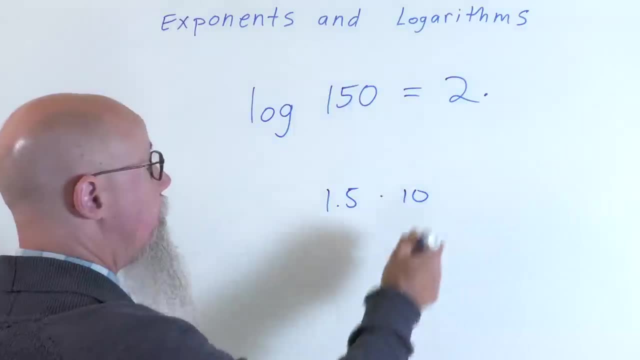 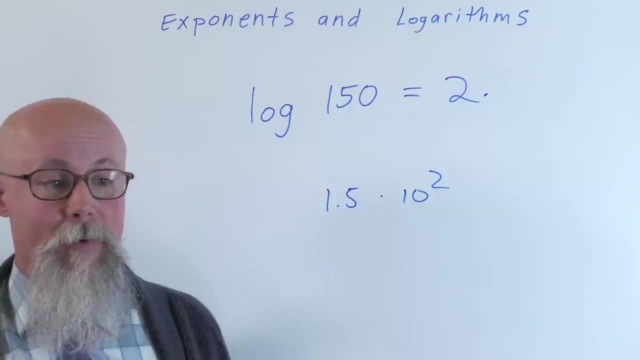 So then that would be, you know, 1.5 times 10 to the second. You see, you know different things that we want to do with converting this for scientific notation, All right. Other interesting things about logarithms: Well, that. 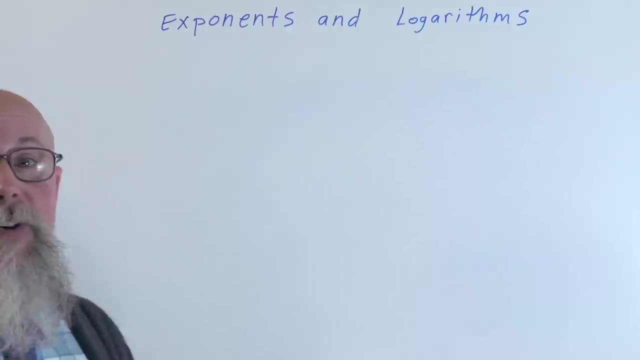 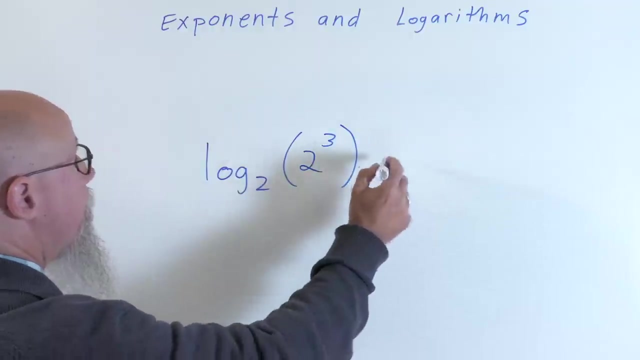 Exponents and logarithms. they're inverses of each other. So if I have, If I have the log base, two of two to the third, Then actually I'm not even going to put it to a definite number, I'm going to call this X, because then any time the answer is X. 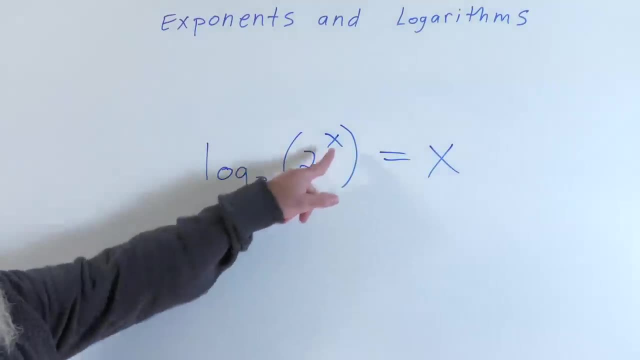 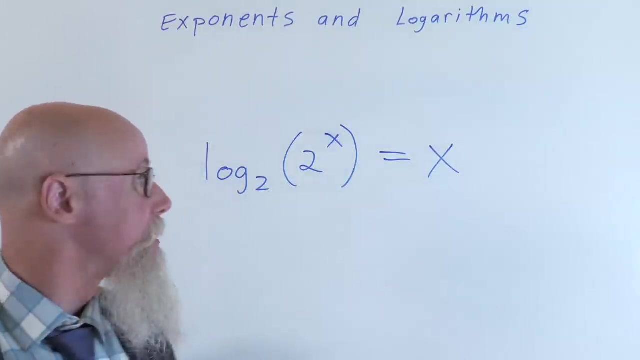 You see, if I take the log of the exponent, Any time you have a function of its inverse, it cancels out to X. Now notice then what we're saying here: the log base two, So two to what exponent gets me two to the X. 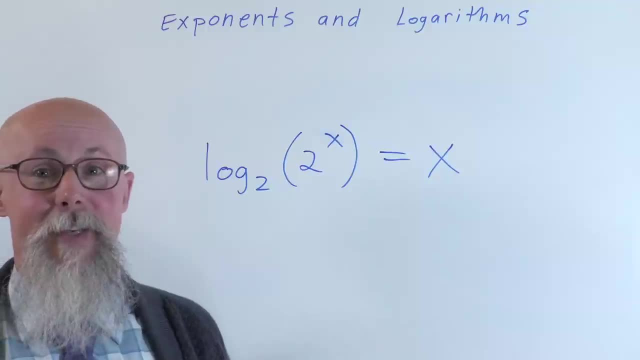 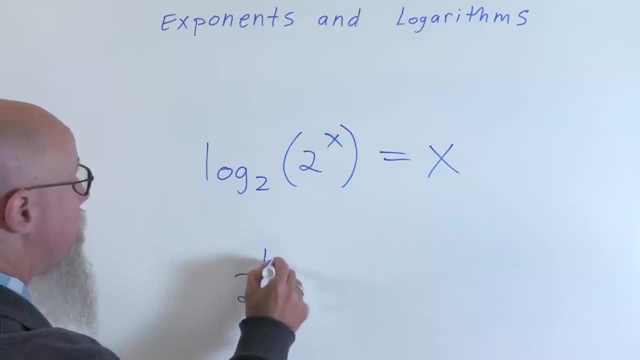 Oh, X is the exponent You know makes sense, And the same type of thing works with. if I have two to the log base, two of X Exponent, Same thing, That's exponent And log inverse. Because, remember, take a look at this: 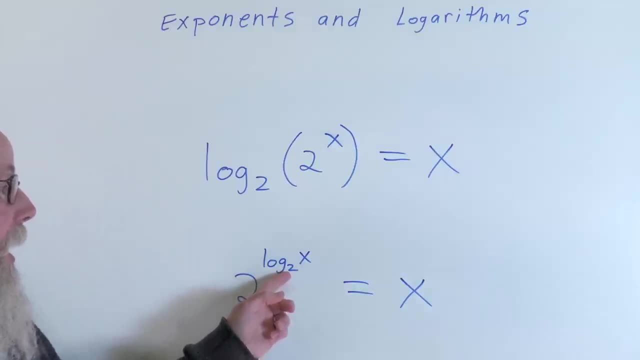 Log base: two of X. So it's two to what exponent gets me X. So remember, any time log we want the exponent Two to what exponent gets me X, And whatever the answer is, it's an exponent And I am then in fact taking two to that exponent. 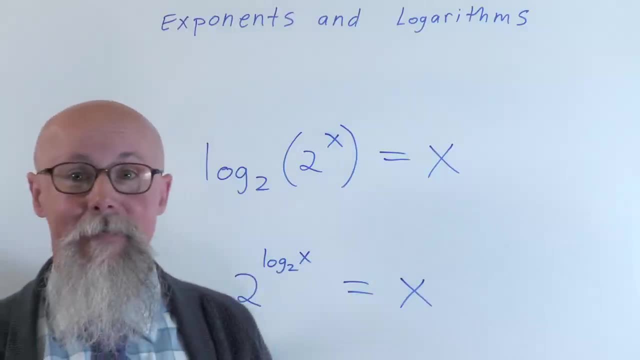 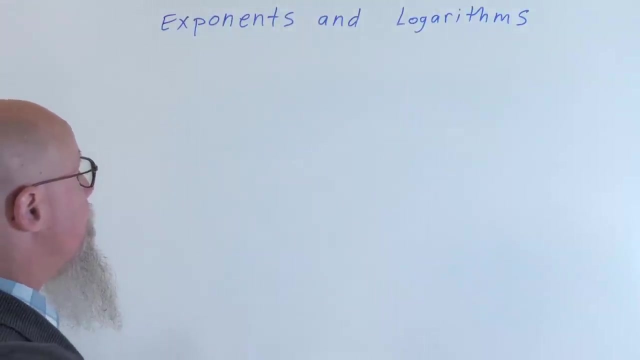 So I would end up with X. So we see, you know we're going to use these inverses, And this is where it becomes very useful. You know, for whatever base I have if I'm solving something, If I have three to the X equals, you know, 25.. 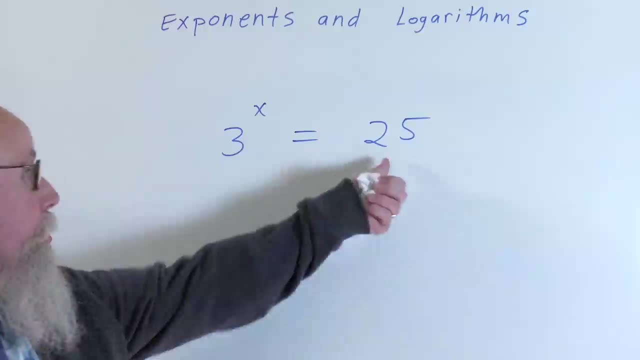 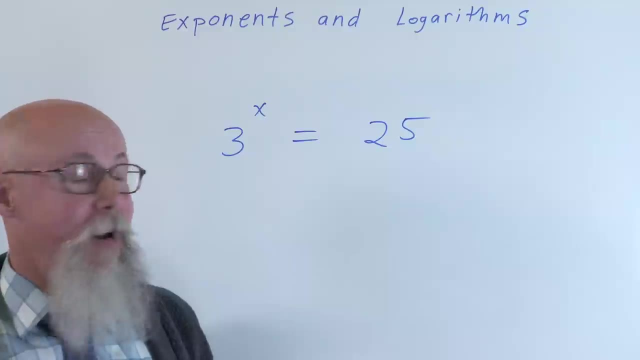 Now, that doesn't work out nicely. If it was 27,. X is three, That's nice, But I know I'm going to do this on the calculator. What am I going to put on the calculator? Well, how can I get? 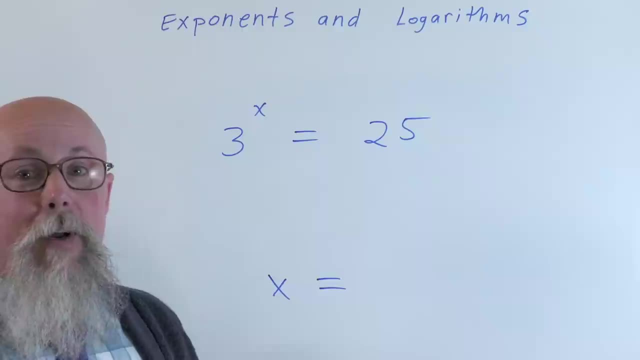 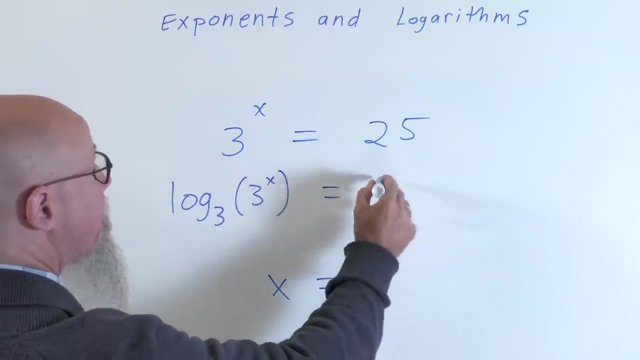 How can I get it to X equals something. Well, If it's three to the X, then if I take the log, The log base three Of this, three to the X, And then On the other side, it's going to be the log base three of 25.. 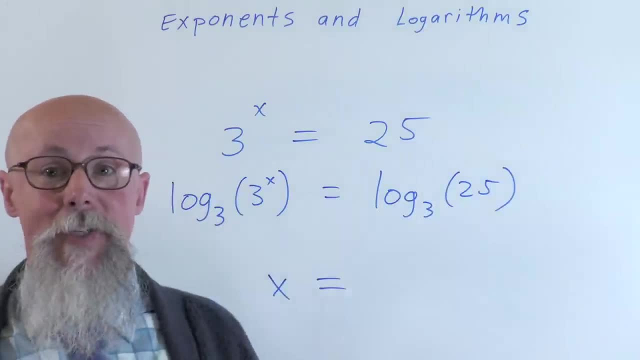 So In algebra, in the things you know, I do the same thing to both sides. What are the things that I can do? Well, one of the things I can do to both sides is take the log of both sides, As long as it's the same base. 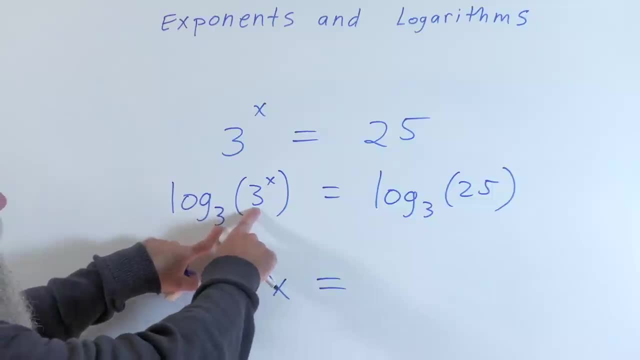 So if I take the log And I pick base three because of this, Because then That cancels down to X- And then over here I have the log, base three of 25.. Which is what I would do in the calculator. 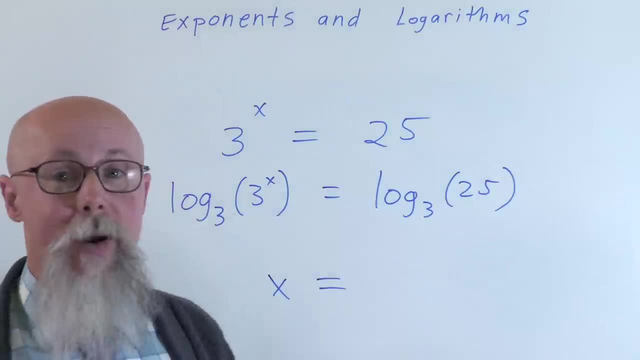 And we'll see in the code. You know we're going to import a library and we'll be able to do this. You know no problem on the calculator Or in the Python code. Now another thing is if you're on a calculator or 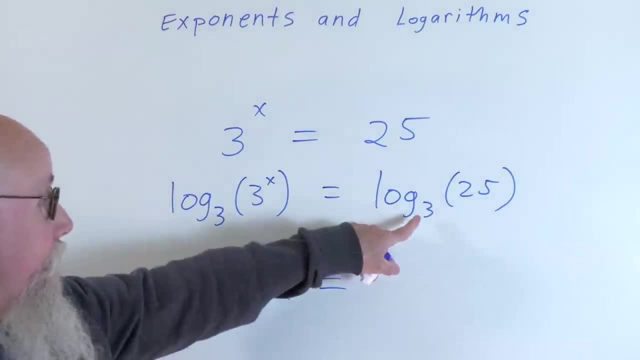 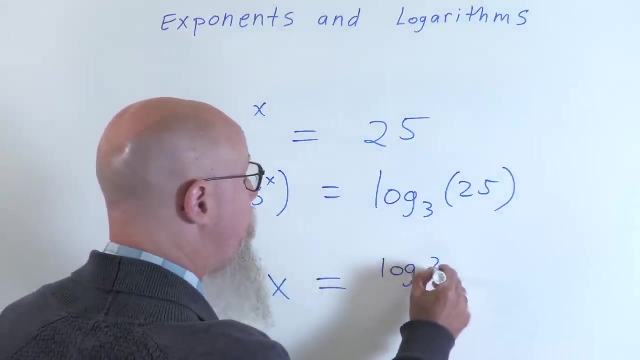 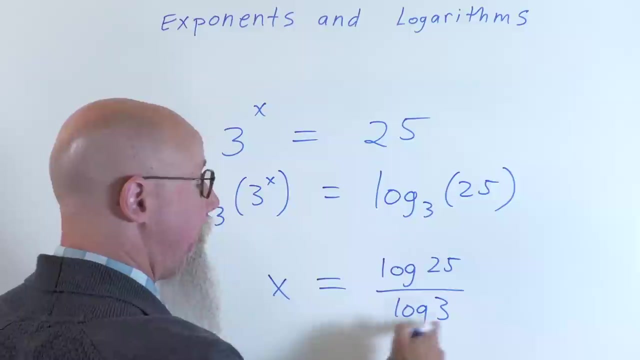 You know you want to do different sort of Python code. I could just do the common log for this. It actually works out. also the log of 25. Divided by the log of three, So the log of this divided by the log of the base. 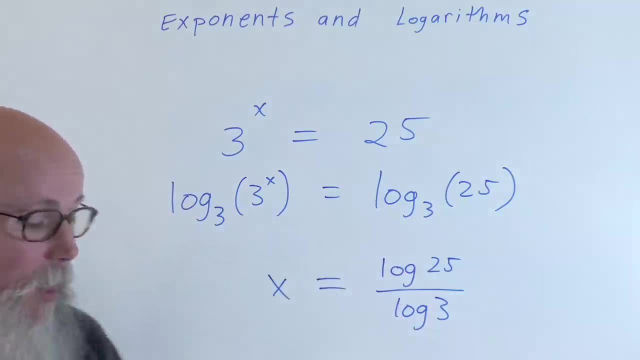 And again It can use common log or whatever I'd want for that. So you know that's pretty interesting. You know what another way that like that works. So change of base formula If you ever find yourself in a situation where you don't have the ability to do the log of any base. 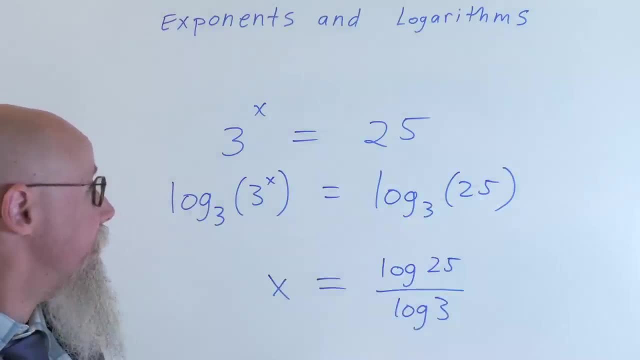 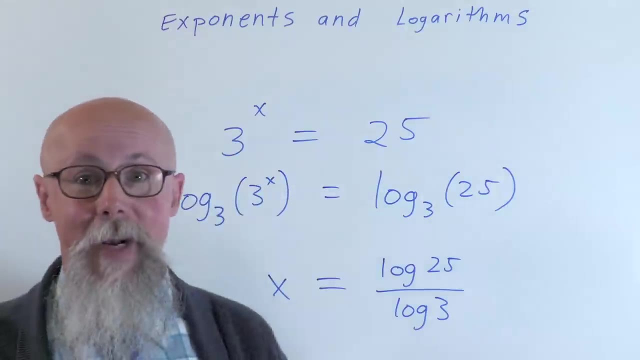 You know you can use whatever logarithm you have and do this. So that's where you know exponents and logs. We use that inverse property when we're solving And that comes up a lot. You know, if I want to look at things, you know things that are growing exponentially. 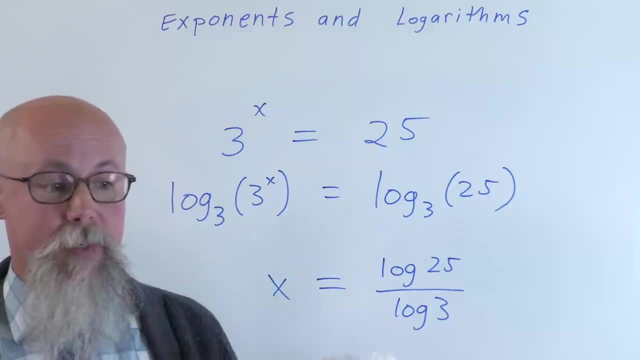 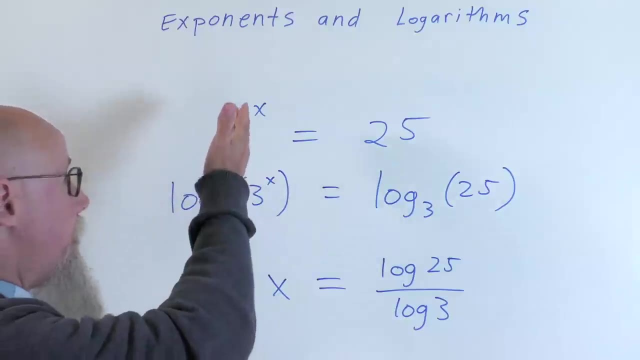 Anything. continuous growth. Sometimes it's, you know, radioactive decay for dating, carbon, All kinds of things. Sometimes I'm in this situation- Exponent My unknowns in the exponent, And so I want to use a logarithm to figure that out. 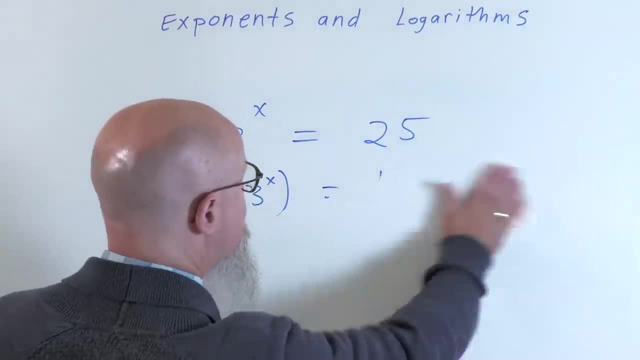 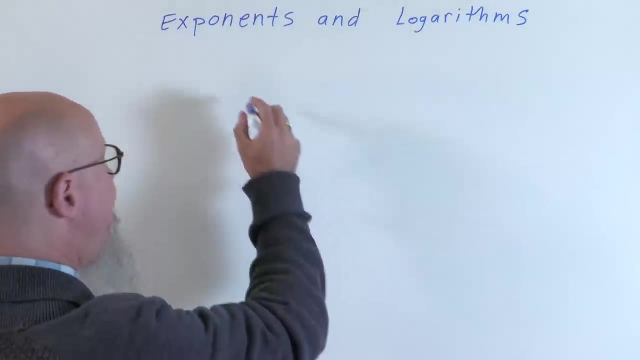 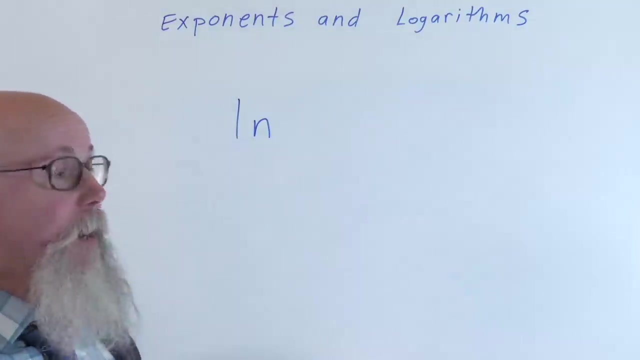 The other log is going to be. So we have all the different bases And the common log, which is base 10.. But then I also have the natural log, And if I was writing this, I'm going to write it as LN. 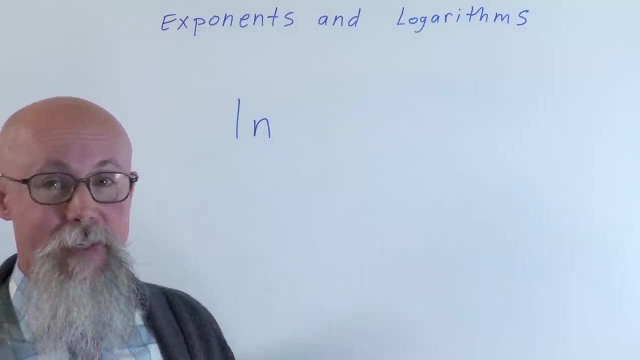 We'll see that a lot of the logarithm functions in Python They actually. If I just say log, It actually goes to natural log, Not base 10.. So that's really interesting. In Python the default is natural log, If I don't put another base there. 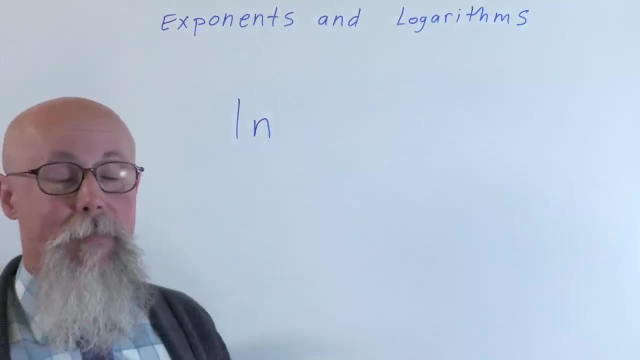 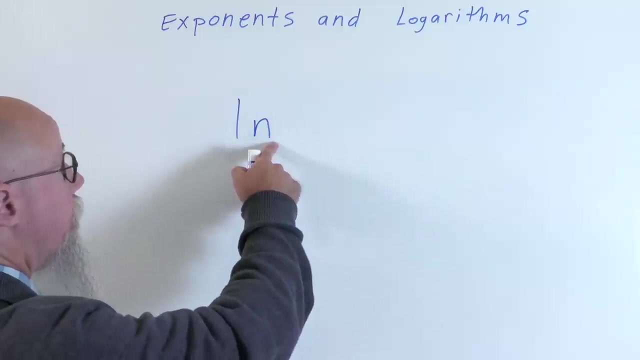 But if I was writing it out, It's LN for natural log, And so if I have the natural log Of Of anything, So The natural log means that it's base E, And So And base E, E is about equal to that 2.71828.. 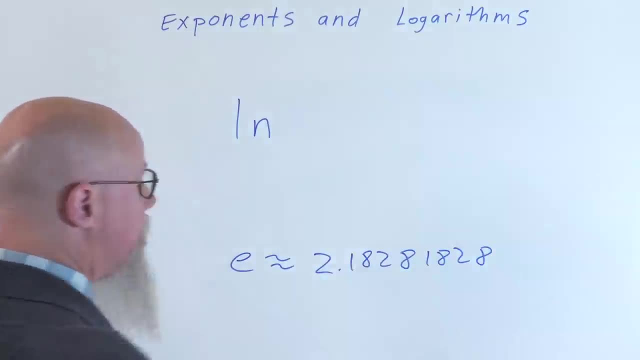 1828. And then after that It's less than five, But then That pattern stops. So, Oh, 2.71828.. So E is about 2.718281828.. And it keeps going. This is used for a lot of continuous growth formulas. 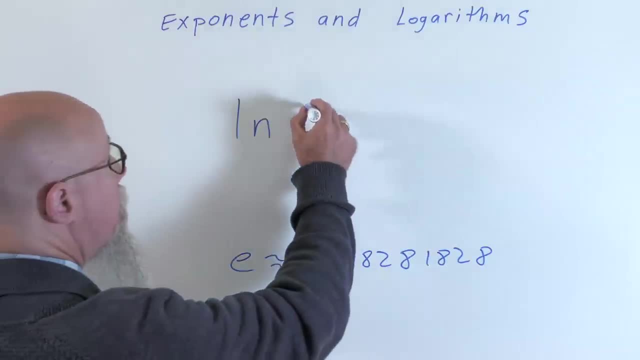 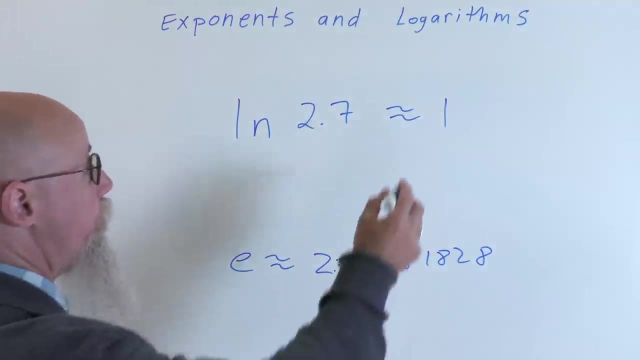 So, If I have, You know, The natural log Of You know 2.7.. Well Then my answer is going to be: You know About one. It's going to be a little bit less than one. 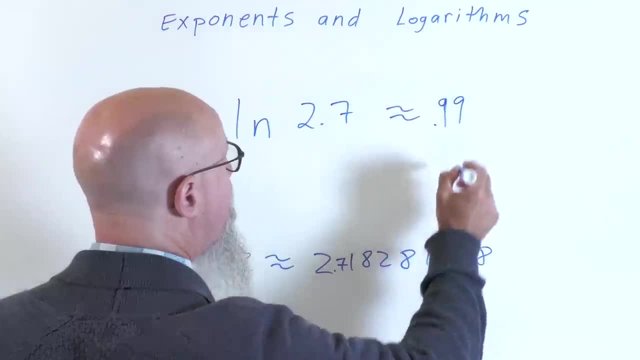 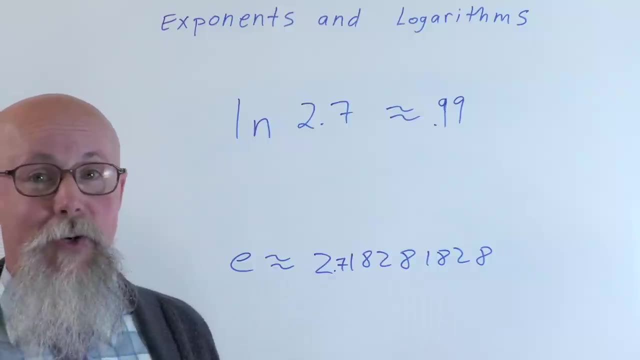 It's like 0.99.. And I can, You know, I can use the natural log for For some other things And we'll We'll see some of the applications of that too When we get to the code. 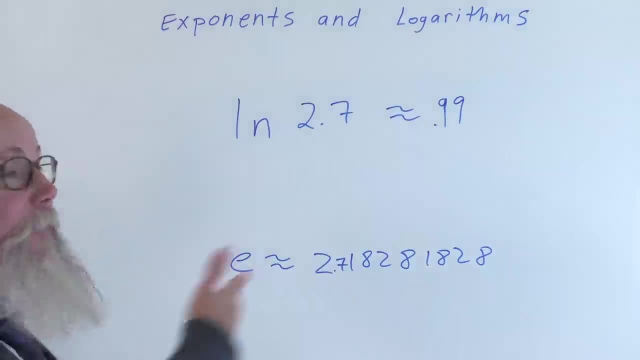 But that That's where. If I have base E, So If If it's base E, I just Make this LN. If it's base 10. I can just write log, And if it's any other base. 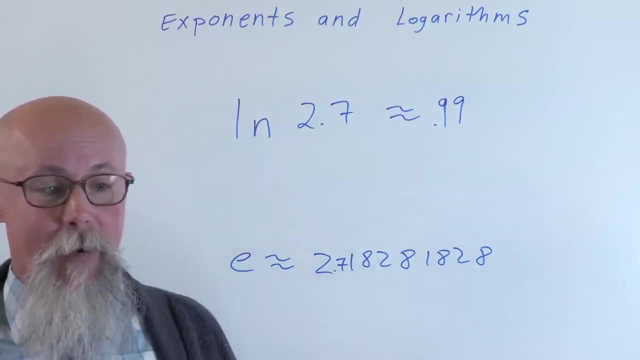 And the bases. We usually want to have them as whole numbers, But if it's any other base, Then I'm just going to actually write the base, So Okay, So We take a look at this, We'll see how. 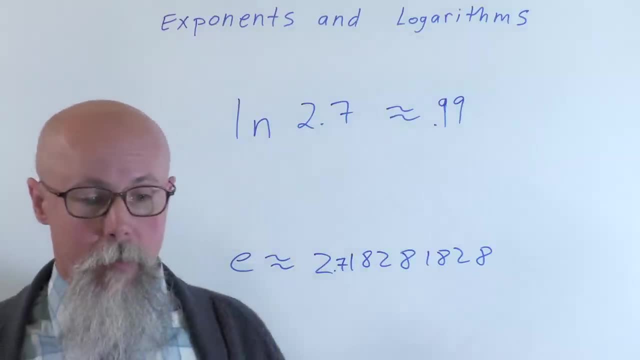 We can actually calculate a lot of this In the code, And that's going to be Pretty useful for some of the Some of the applications we have. So Let's take a look at the code. So, When Using logarithms, 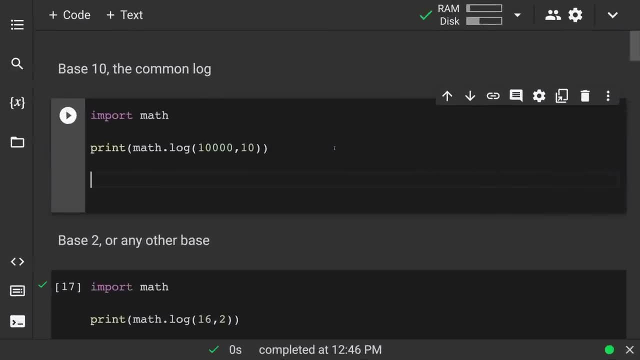 In Python, We'll just Import The math library And Now we have Math Log. There we go Math Log. So When We Use Math Log And it takes two arguments: The number, 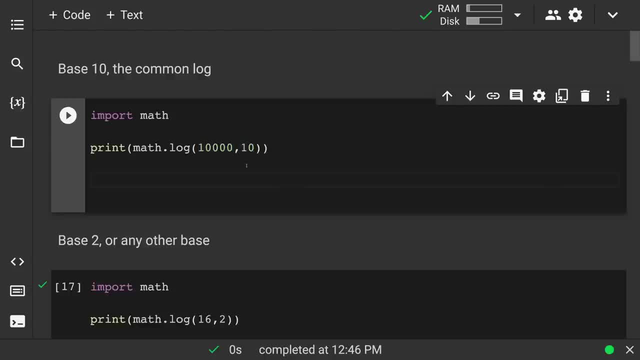 And then The base. So This is Math Log Of ten thousand Base ten. So When I run it, There we go, It'll be four. This works out nicely for Things that we know Are going to be. 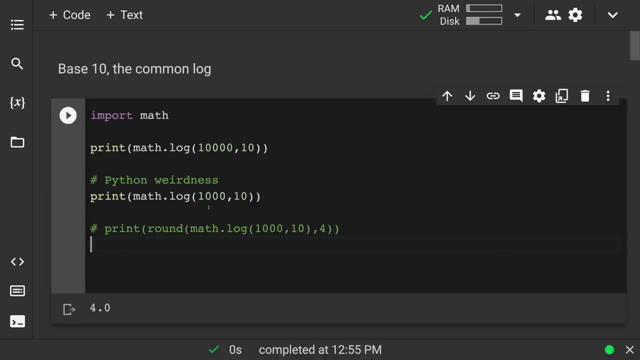 A nice integer. But I also want to show you That Python Weirdness. Sometimes, Even when you think it's going to be a nice integer, Math Log Of a thousand Base ten. So I expect this to be exactly. 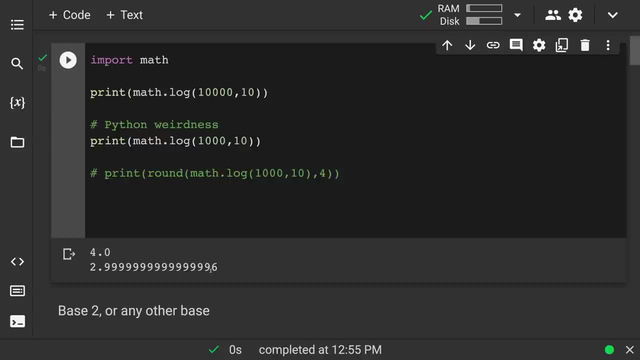 Three, But when I run it It gives me this Long Decimal. So Any of these, Even when you think it's going to work out nicely, Just the way That this Works Behind the scenes- You might want to. 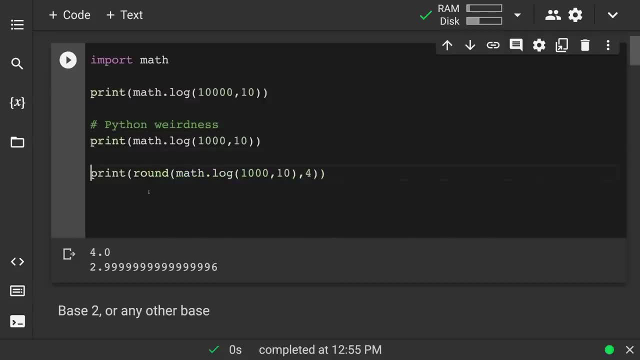 Just Build in A rounding Function Here. So I'm going to round All this Math Log Of a thousand Base ten And I'm going to round all that to four decimal places. So You just might want to build. 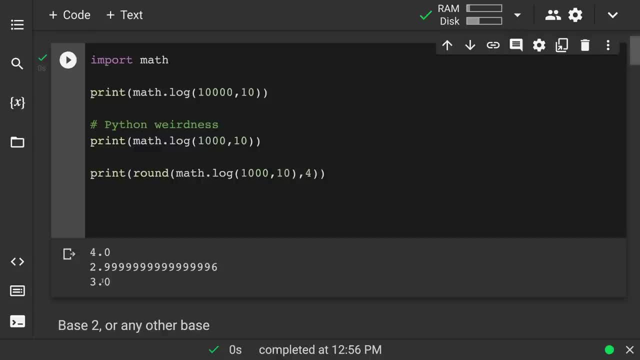 Build that in So That way You're going to get that answer. And notice, I still Said four decimal places But because it worked out Not Rounding, Not needing Decimal places, It didn't have to give me. 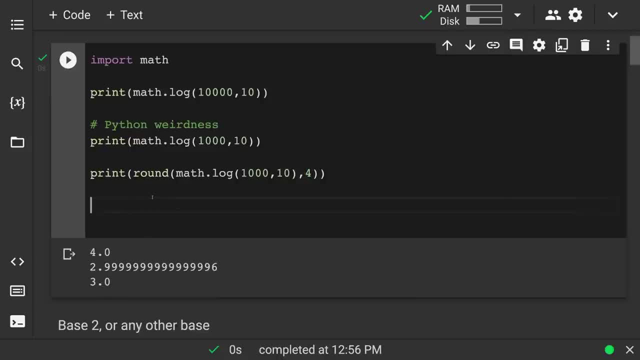 Like four zeros After the decimal. There we go. So That That's just The usefulness of it, That It It's just worth it. Build the round function there, All right. So That said I. 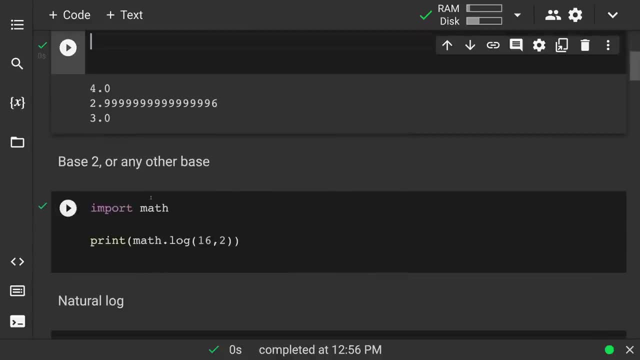 Have a few of these, that I don't have the round function, Just to show you what the exact answer might be. So If I have Base two, There we go Again, Import math And then we're going to do math. 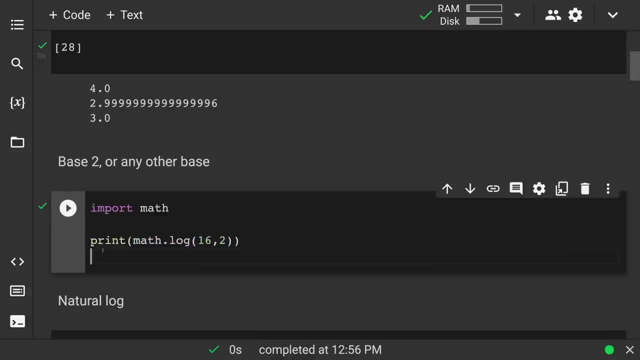 Log, In this case Sixteen Base two. So When we run it It's going to be four And I don't have the log In there. So If I have something like Fifteen Base two, 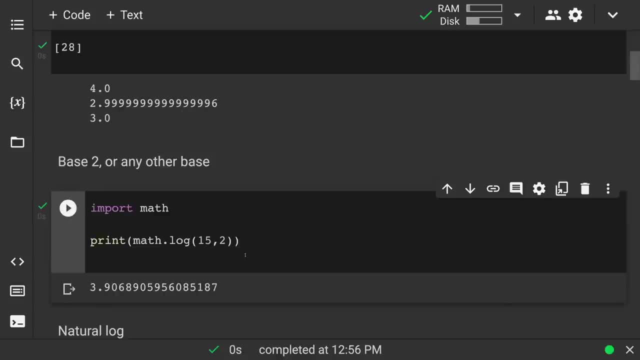 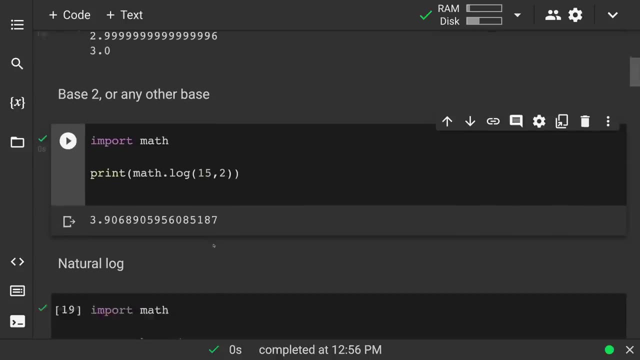 I don't have the rounding. So You see It, If I have All these decimals for For something, It will give you that. But there you go, Just Whatever the number is, And then Base Natural log. 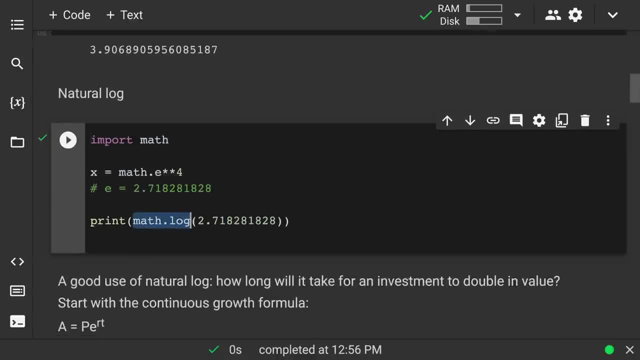 I'm going to import math again And Notice, here I can just do math Log Of a number And If I don't give it that second argument Of What the base is, It'll default to natural log. 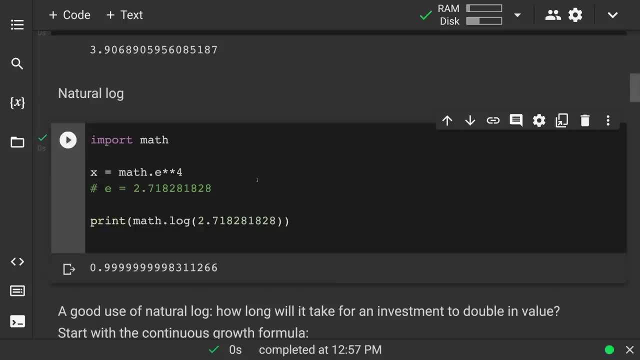 And E Is about Two point seven. So If we We do this, We see You know Now. What I also want to show you Is As We were talking about before, So Math dot. 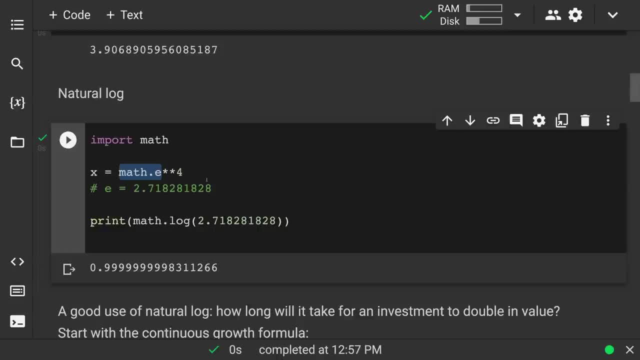 E. If I just want to use E For anything, Math dot E Is going to be the most exact. You know It'll give you All those decimal places You don't have to. just You know, Guess at it. 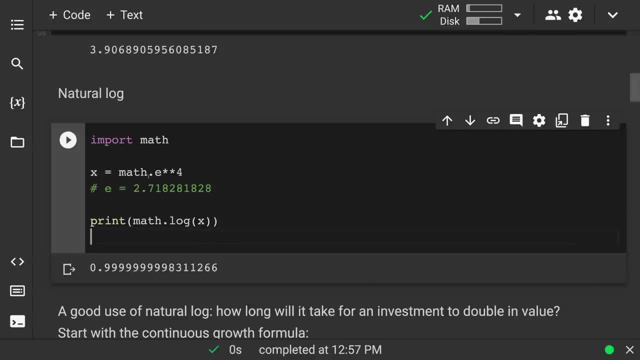 But also E to the fourth Then, And I store that as Variable X. So If I have Four- Because The log Of that exponent- Or If I have E to the third, The answer's. 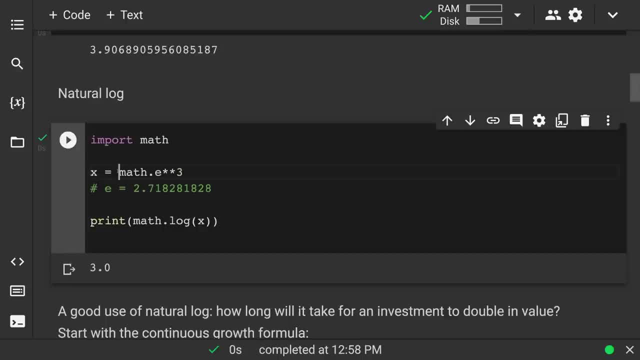 Three. So You know, If I Use that Math dot E To get the most exact Approximation of E And then Log Without The other Argument, Then It Will cancel out And that'll. 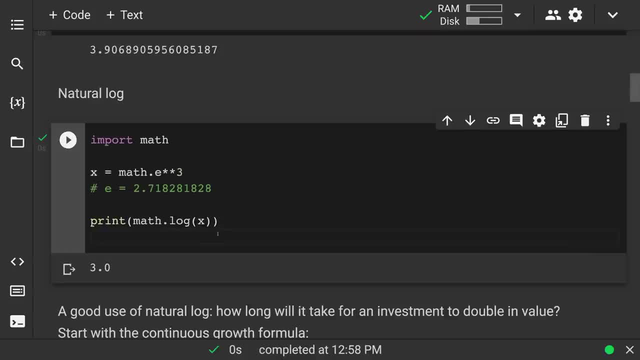 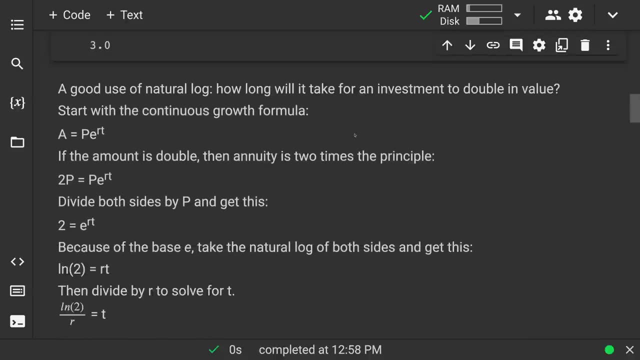 That'll work out the same way If I did Like N. You know That works too, So Just Just To show you this. All right, So Other Good Uses Of Log Or: 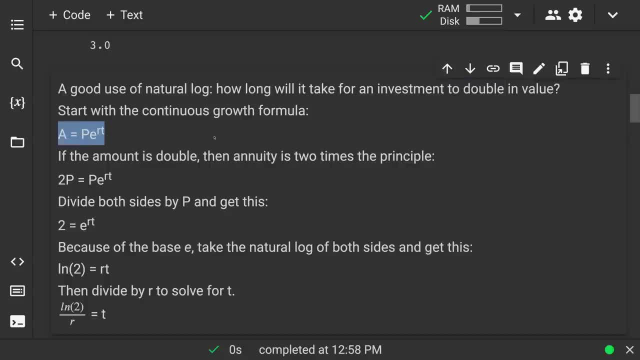 Especially Natural Log Answering The question: How Long Will It Take For An Investment To Double? Then Whatever I Have For P Doubling Would Be: 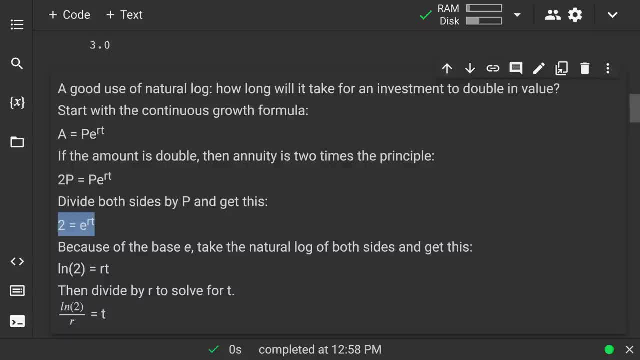 Two P, Whatever The Number Is, So I Can Divide Both Sides By P, And Then I Get This Natural Log Of Two And On. 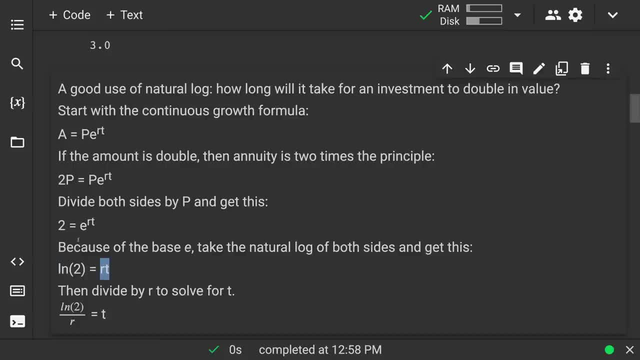 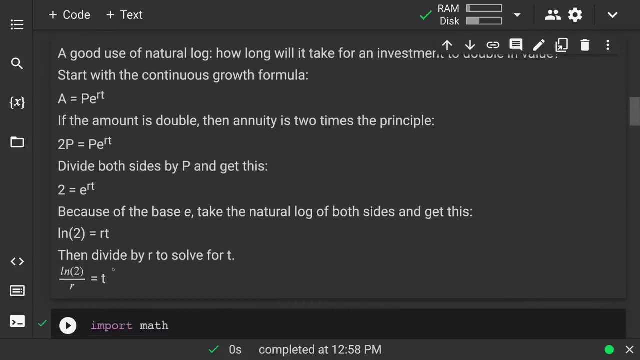 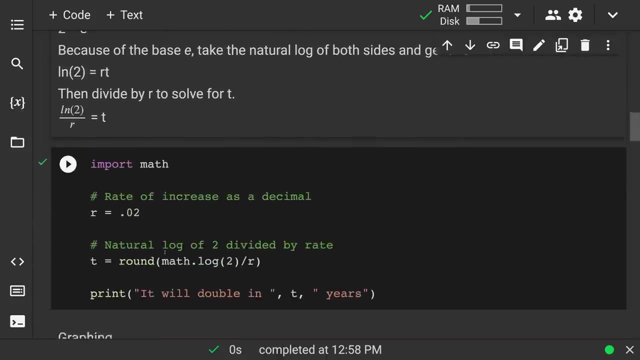 The Right Natural Log Of E To The R T, As We Just Saw, Is Going To Be That Exponent. So That's Why So We? 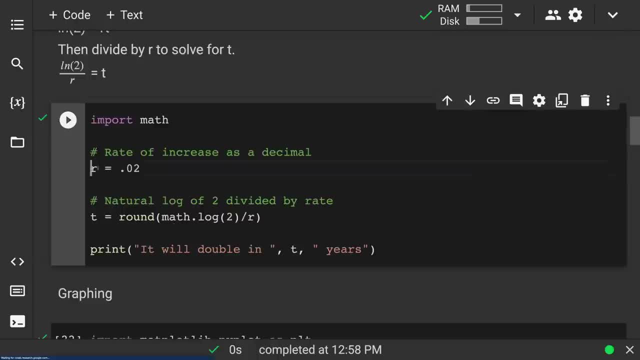 Can Just Put This In Some Code. I'll Just Define R As The Rate Here. You Know, Two Percent, You Know Sort Of Like A. Low Inflation You Get To Be Thirty Five Years. So If Something's Increasing At Two Percent Thirty Five Years From Now, It'll Be Double. 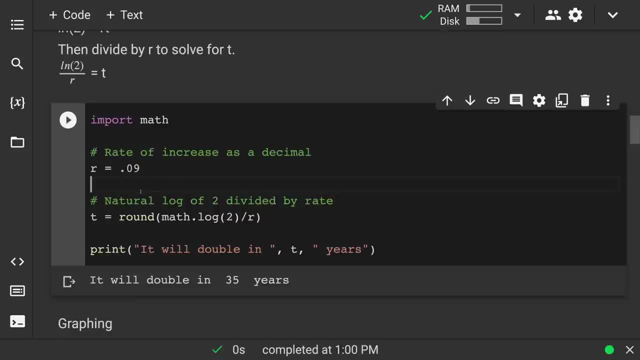 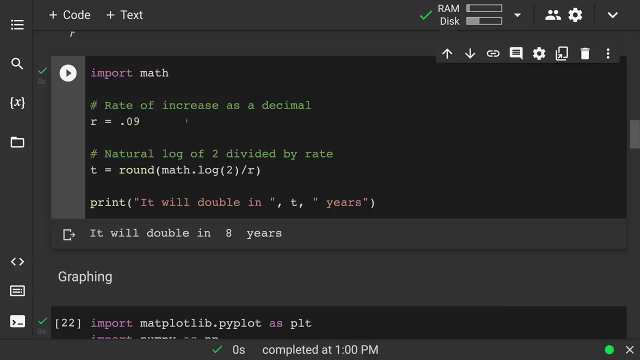 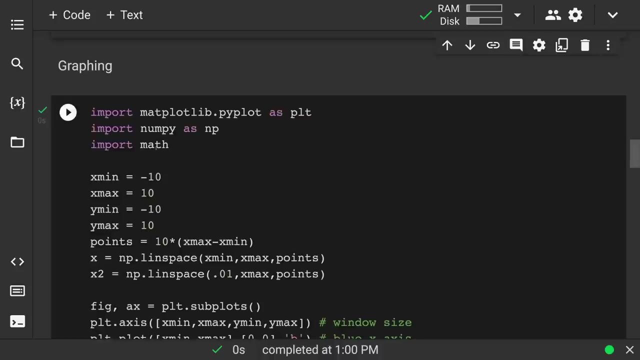 And, Like I Said, As A Low In This Case Eight Years. So There We Go. So You Know, Some People Might Make That Determination. 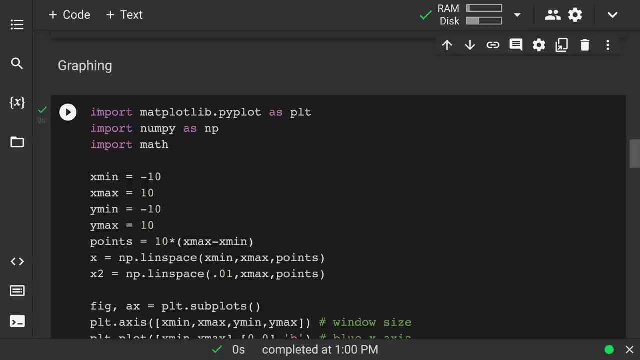 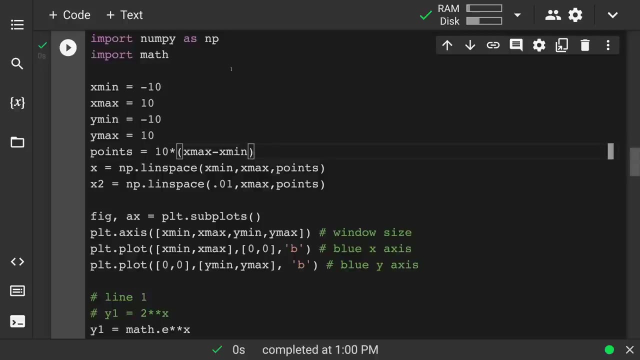 For What They Invest In. And There We Go, Answering That In X Max Set The Dimensions Here, And We've Done This Before When We 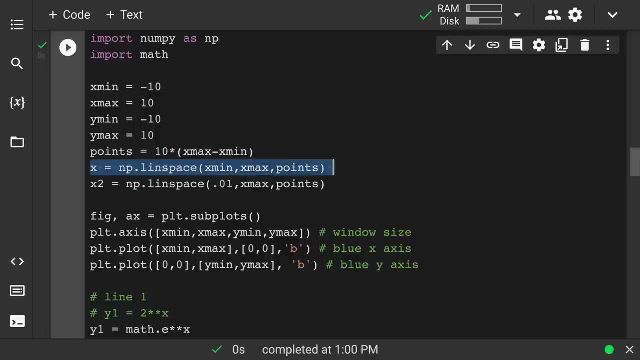 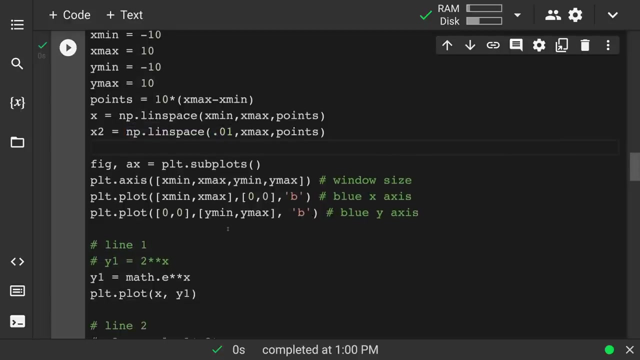 Use Num Pie. I Need The Note, I Need This, The Number Of Points Here- And I Don't Want To Go Down To Negative Ten. 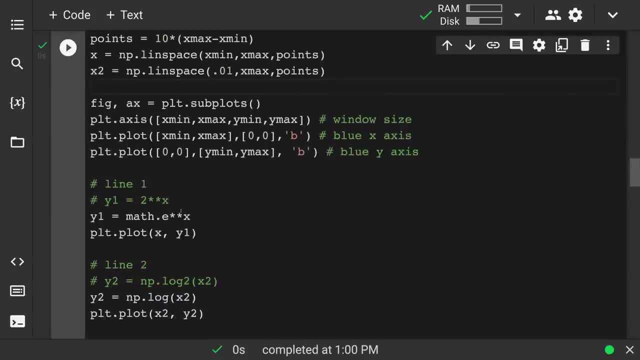 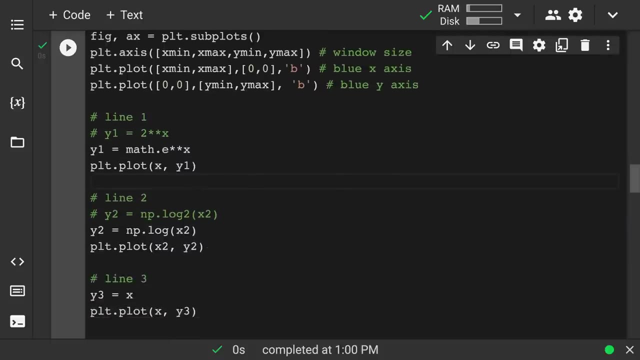 I Want To Start At Point Oh One, And We'll See That In A Second, And Then Again Set. So Then, If It's Either The 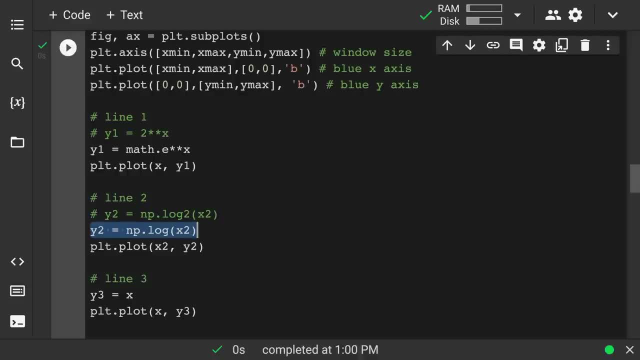 X, I Want To Do The Natural Log And So Notice It's Log, And I Didn't Use The Math One Here. I Wanted To Start. 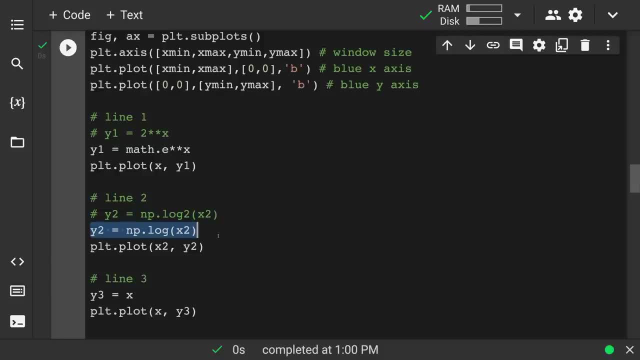 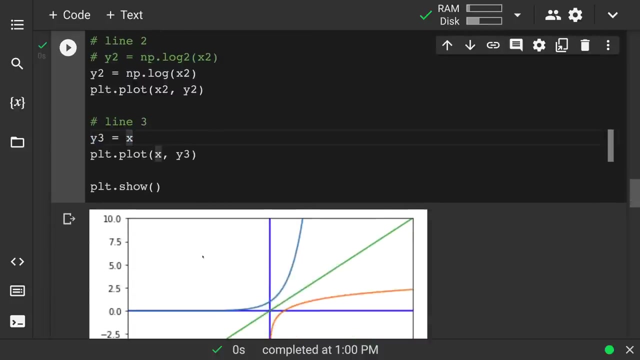 At Zero. So I Didn't. This Actually Would Give An Error, But It Would Still Graph It, Just With That Error, And I Didn't Feel. 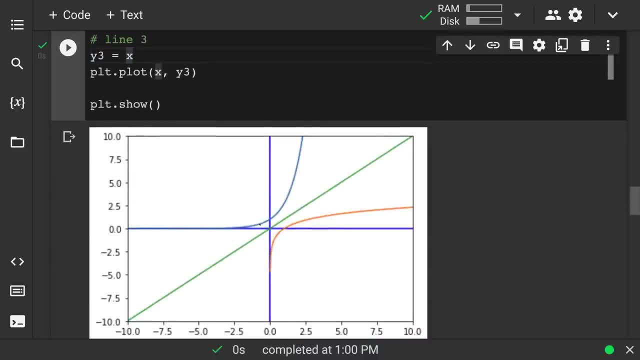 Like Seeing And This Blue Line That Curves Upward- That's The Exponential Function- And Going To The Left It Actually Doesn't Really Touch. 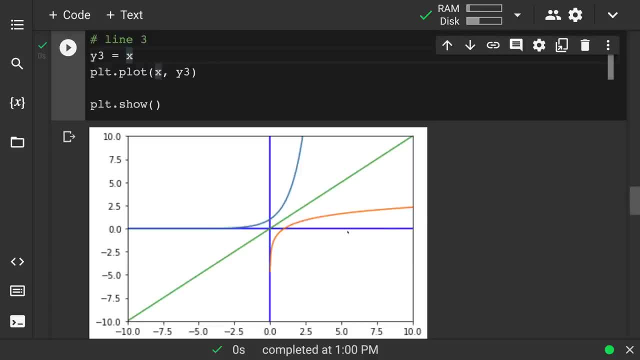 Zero. It Just Gets Really, Really Close Beyond X, Especially As It Goes On And On. And Then The Green Line Is Y Equals X. So 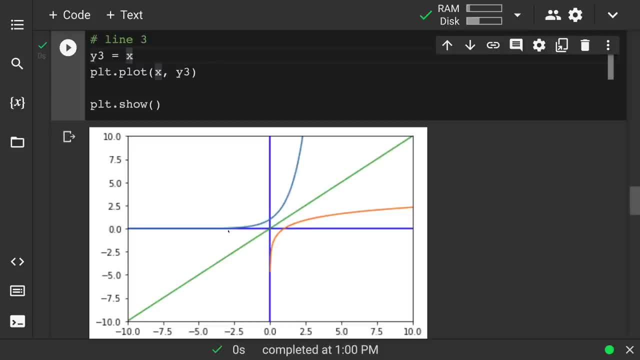 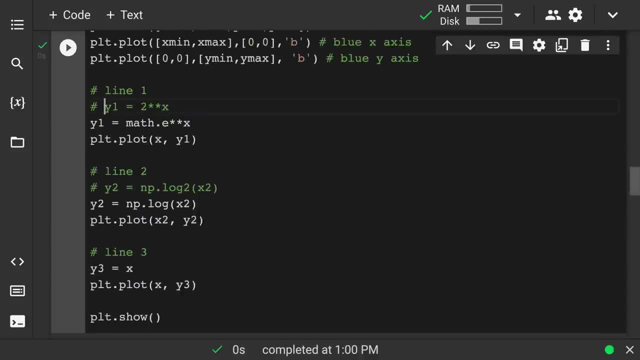 If It Looks Like These Are Mirror Images Of Each Other, Thing That I Have Two To The X And I'm Going To Use This. 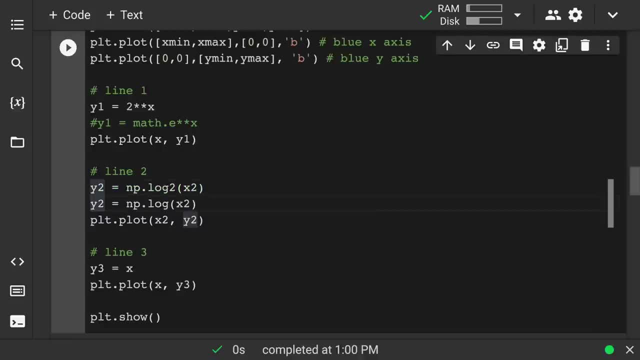 And Comment Out This Other One. So Instead Of E To The X, If I Draw The Line, Is A Log Two Is Log Base Two. 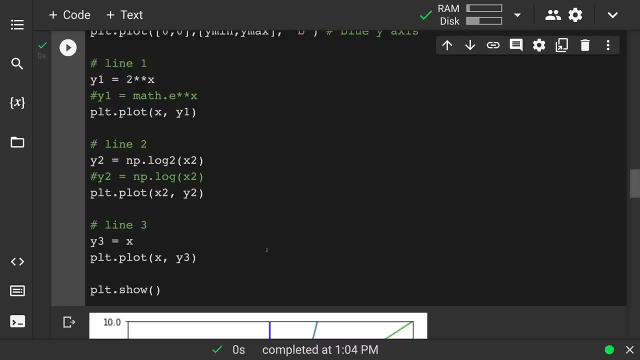 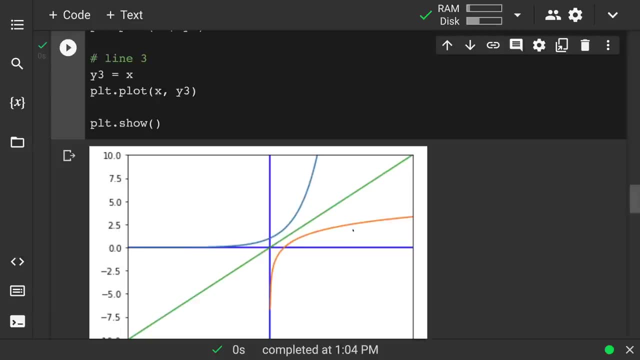 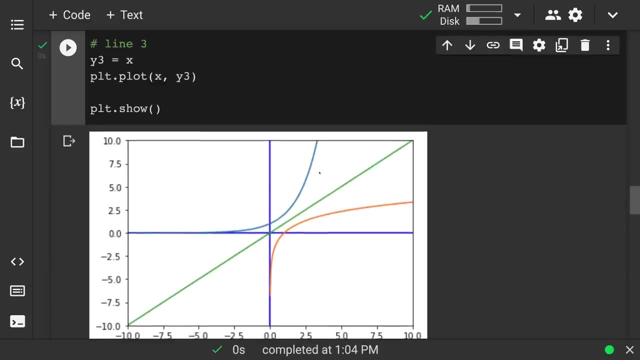 And Then There's Log Ten. Those Are The Main Ones You Want To Be Able To Use. There Is, So I Would Say How They. 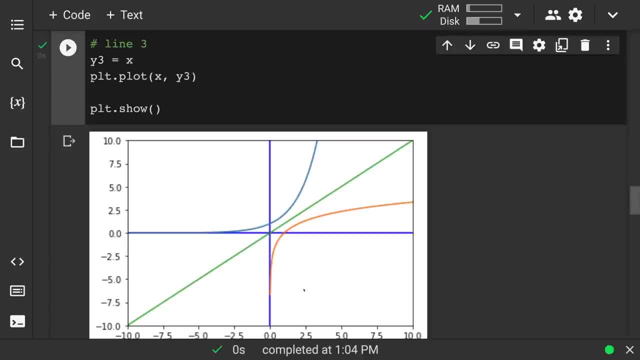 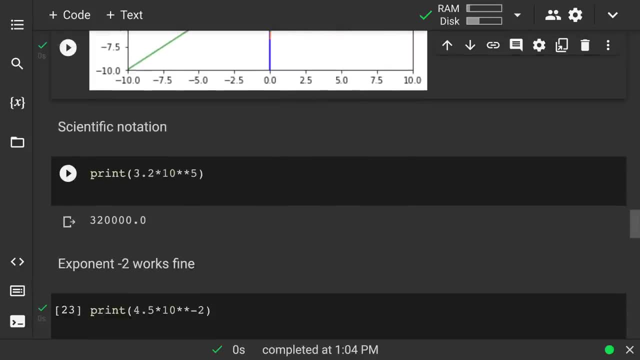 All Kind Of The Same. You Know, Exponential Log, Rhythmic Y Equals X. There We Go. So We Use These As Some, And Here, 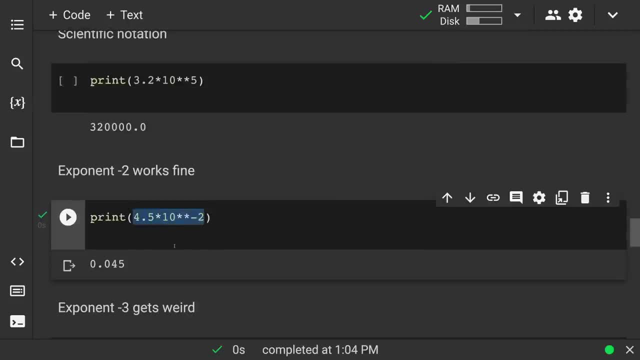 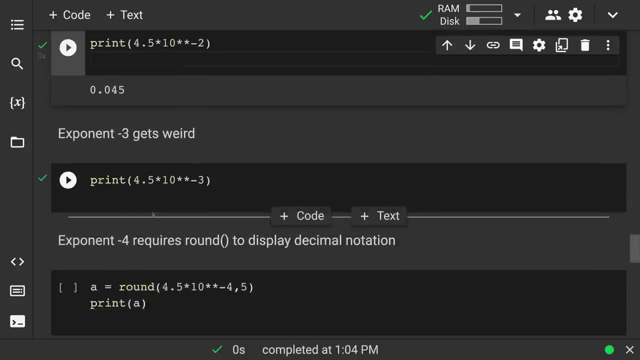 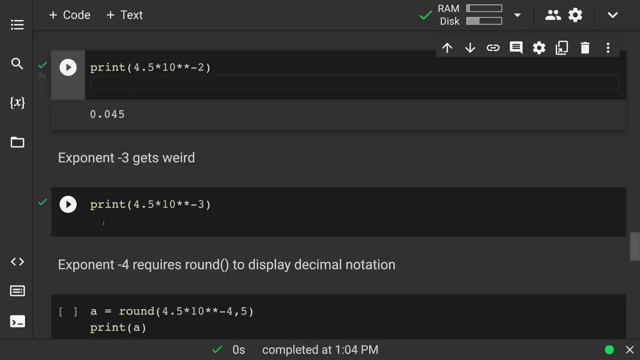 I Have It As A Negative X Minute. Four Point, Five Times Ten To The Negative Second. There We Go, And You Might Be Wondering. 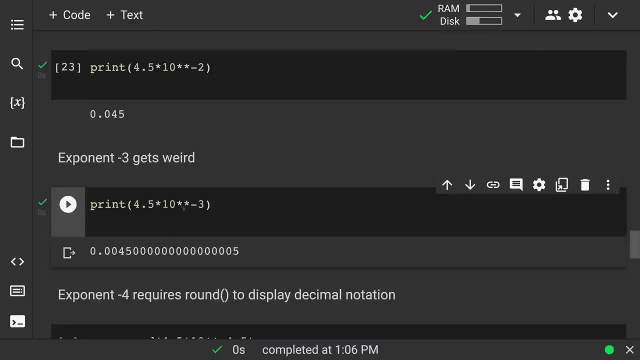 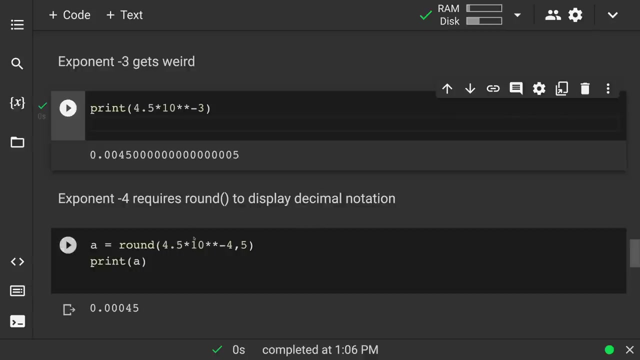 About That. You See Just The Way It Works Behind The Scenes. The Negative Three. We Would Think That It Would Stop There And That Be. 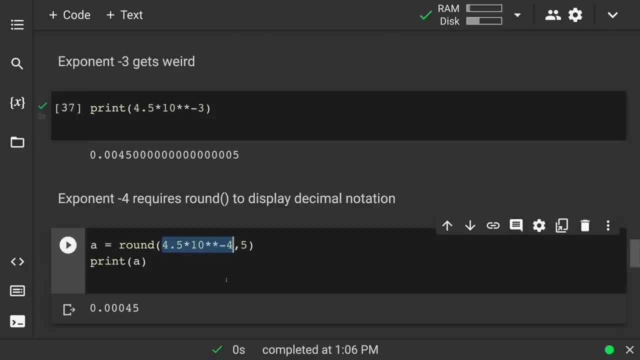 Fine, But It Gives Four Point Five Times Ten To The Negative Four, And I'm Going To Round It To Five Decimal Places. So If 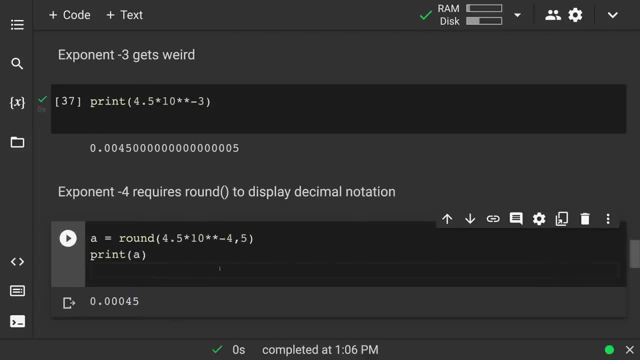 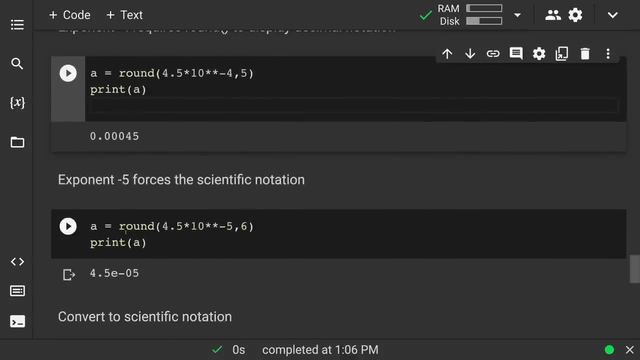 I Have A Negative Exponent, Let's Say Negative Five And Greater. It Forces The Scientific Notation. So As Much As I Want To Say, 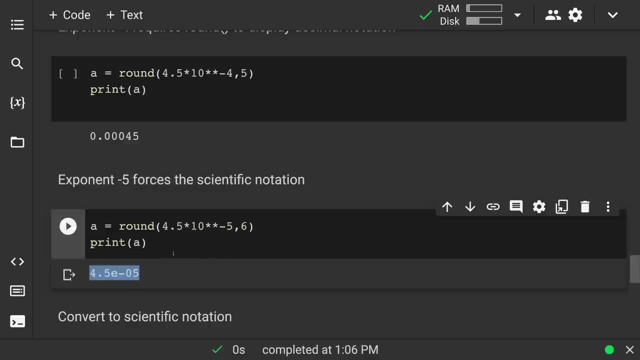 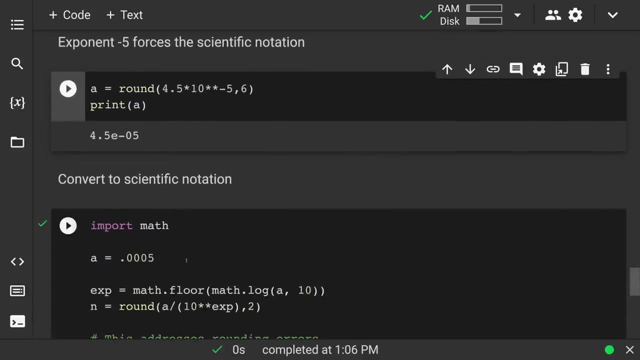 That I'm Just Going To Print This Out. I Already Have It In Uses This, And A Lot Of Calculators Use That Notation Also. 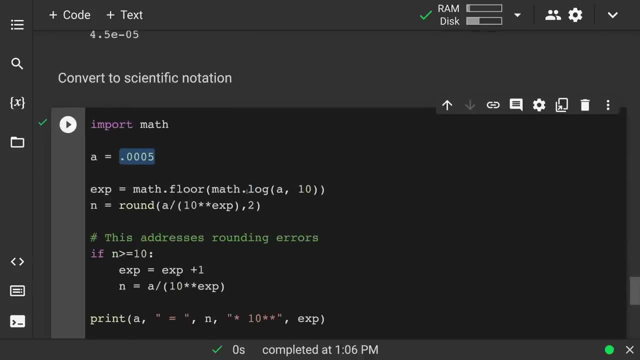 We Can Convert Something To Scientific Notation If I Take This, So I Want To Get The Number Zero One. It's Not Going To Work. 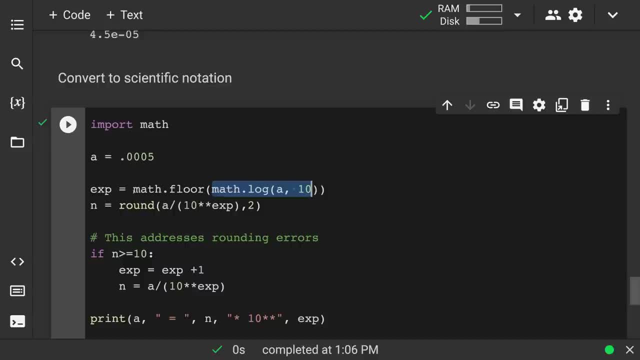 Out To. It's Going To Be Like One Point. You Know It's Going To Be Like. This Is Four Decimal Places Going To Negative Four. 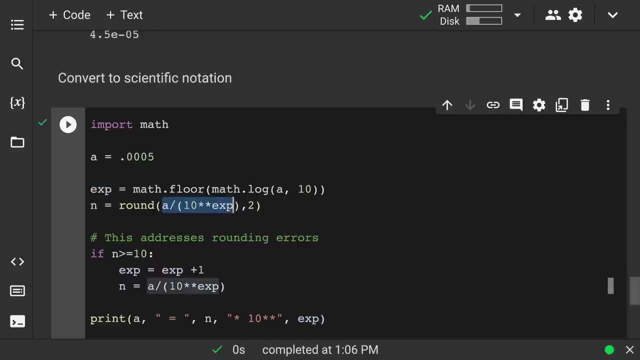 And Then If I Take In, I'm Going Around That Ten Divided By That Exponent, And This Formula Also Works For Larger Numbers To. 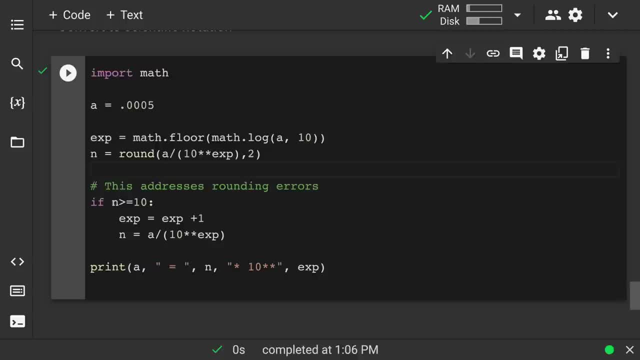 But If You Think That You Are Going To Be, To Be In This Case, Then I, Then I Want To Make Sure That I Still 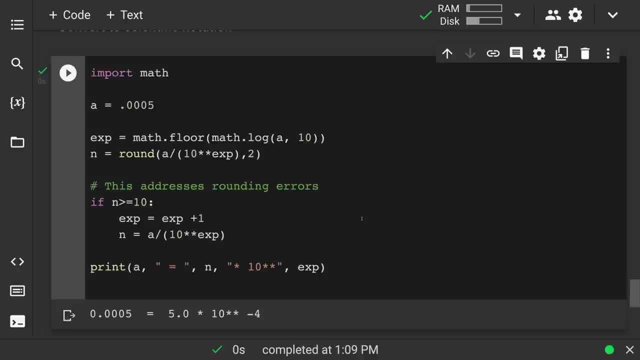 Get True. Scientific Notation One Is You Point Zero, Zero, Zero Five Equals Five Times Ten Of The Negative Four, And Then This Should Work. 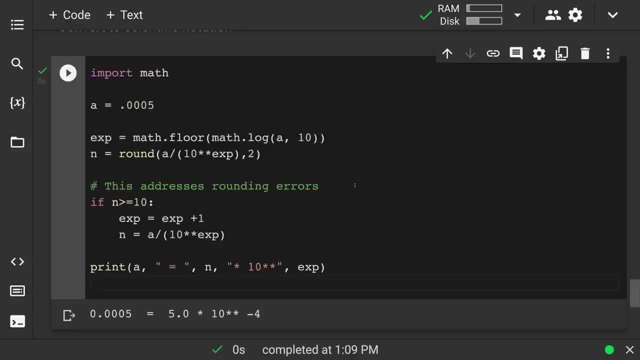 For All Kinds Of Other Exponents Converting Scientific Notation, Converting To And From Scientific Notation. So These Are A Few Applications Of Logarithms. 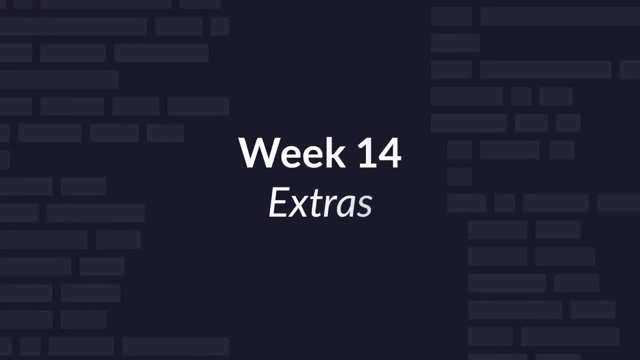 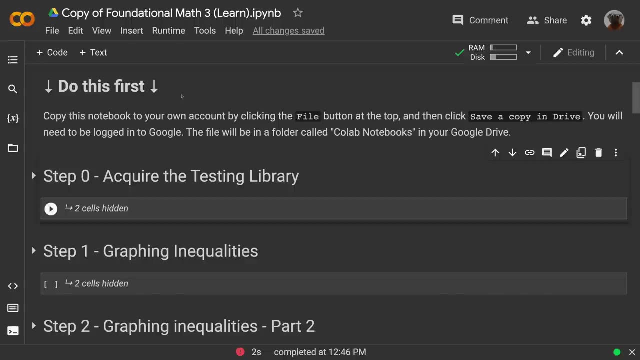 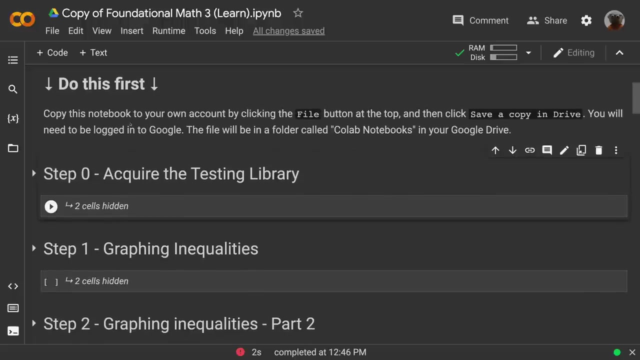 And I'm Sure You Will Find Even More. So Make Use, Make Use Of This. You Are Going To Make A Copy. First Of All, 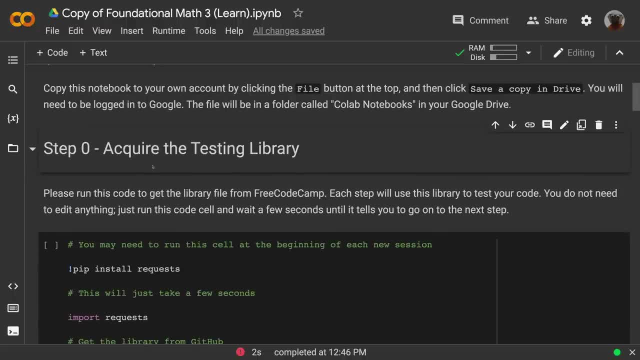 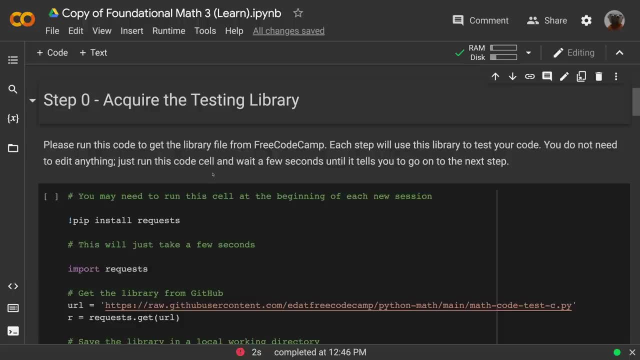 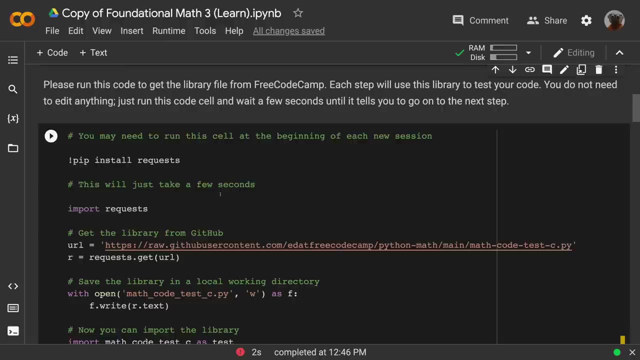 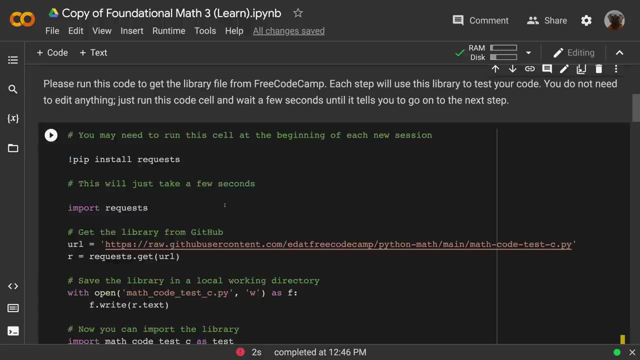 And Work Through This Whole Notebook, Make A Copy, Put It In Your Google Drive And Then, From Your Virtual, Your Own Library Hosted On 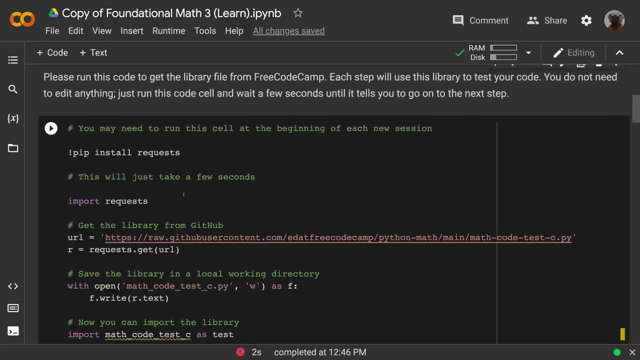 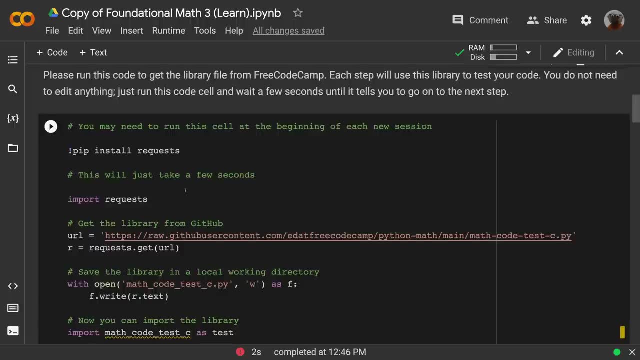 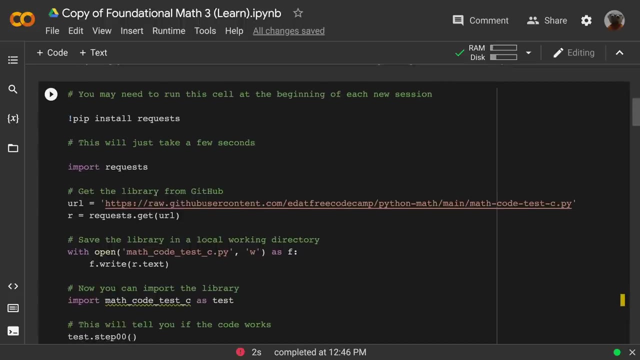 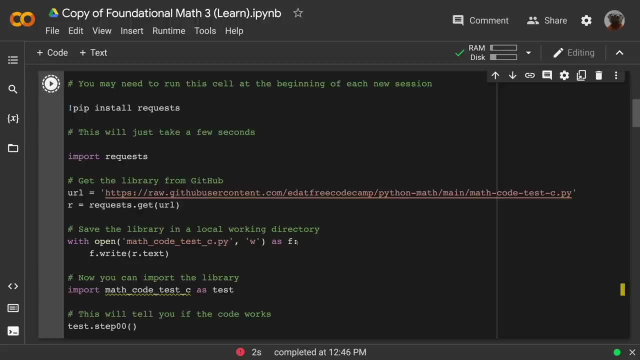 GitHub And Use That, Import That Into Whatever Notebooks You Want. So You Know, As We Get Through This Course, You Know You Can Get. 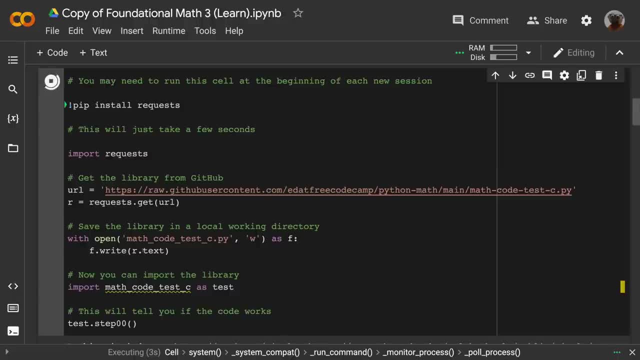 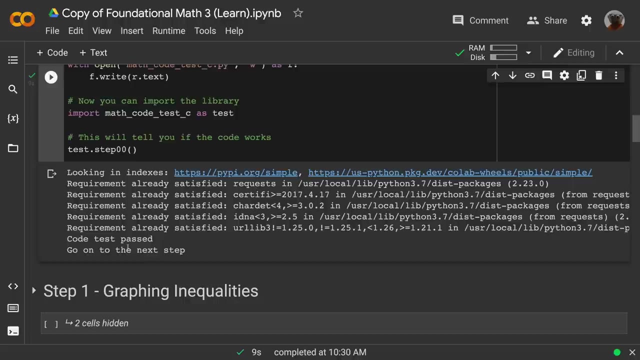 The Library. Take It As As A New File Locally, Here Behind The Scenes. We Won't Have To Worry About It And It's Imported. 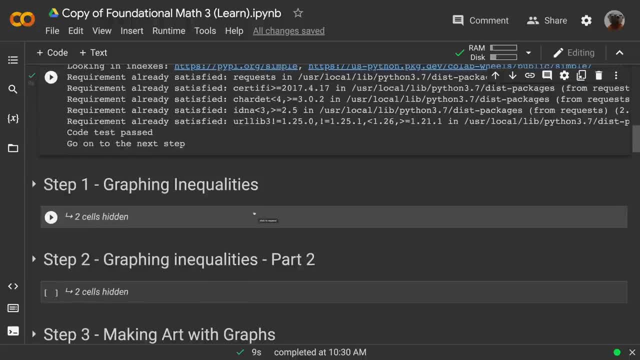 There We Go And Run Time. It Times Out, You Know, Twelve Hours Consecutively At The Most, Or About A Half Hour Of Inactivity. 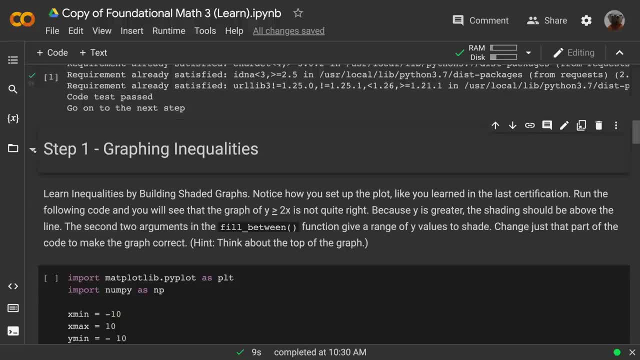 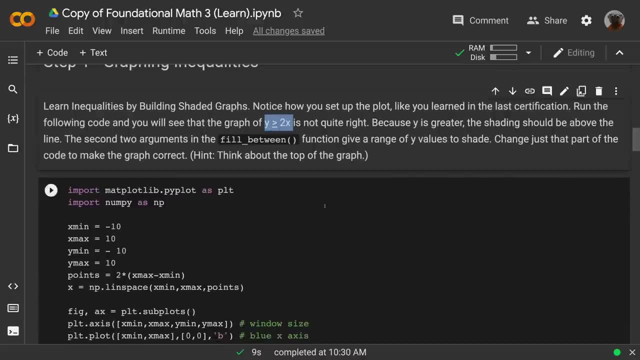 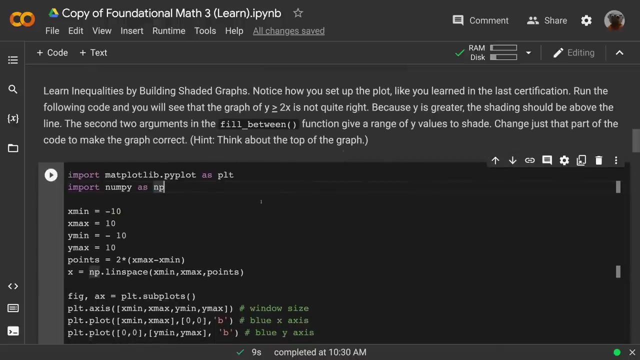 So You Just Get In The Habit If You Is Greater Than Or Equal To Two X. Well, If I Have, Then If I Can Grab. 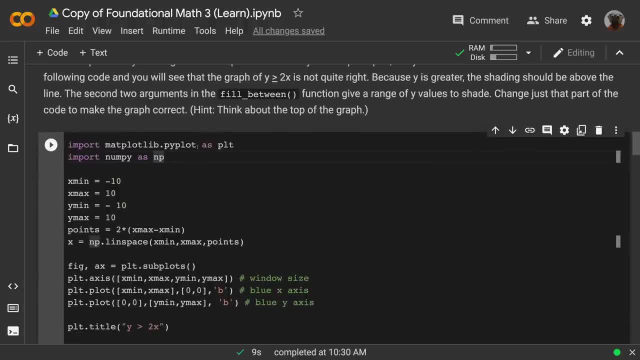 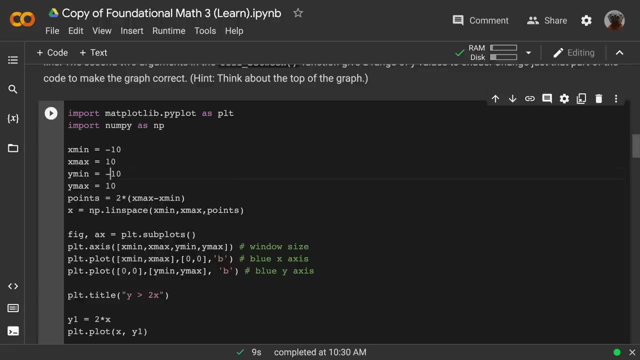 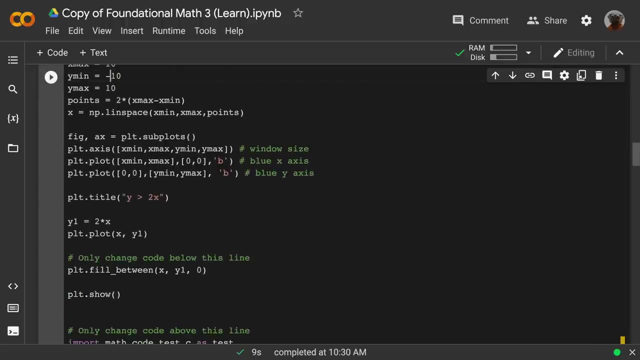 The Line. But How Do I Shade That? Well, We Have This Window, Like We Were Doing Before. How Many Points, You Know? Numpy Linspace. 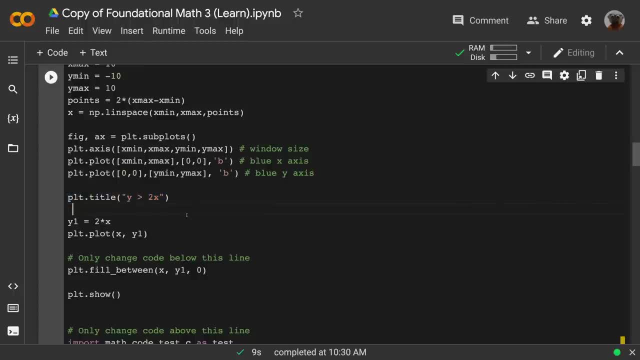 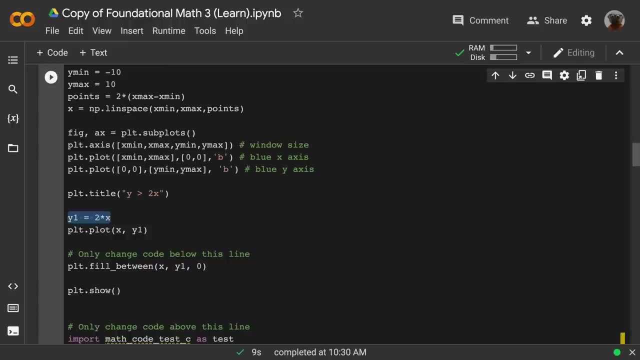 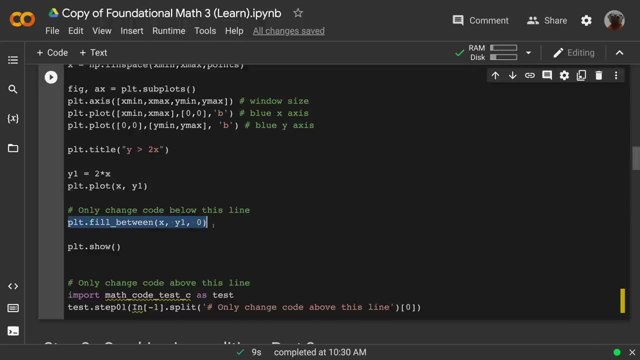 Give Our Points, Setting Up The Graph- All This Is Very Similar. This One Got A. There We Go. Here's The Code: Change And Remember. 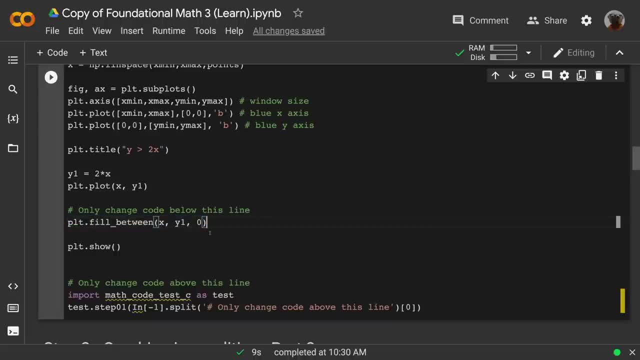 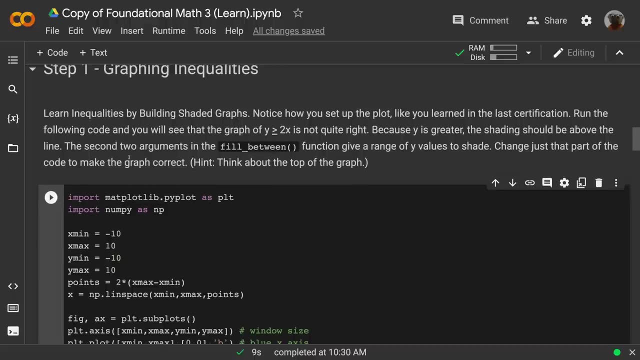 This, We Have Plot These Two And Then We Have This Third Argument. So If You're Working Through This And Our Insight About This, But 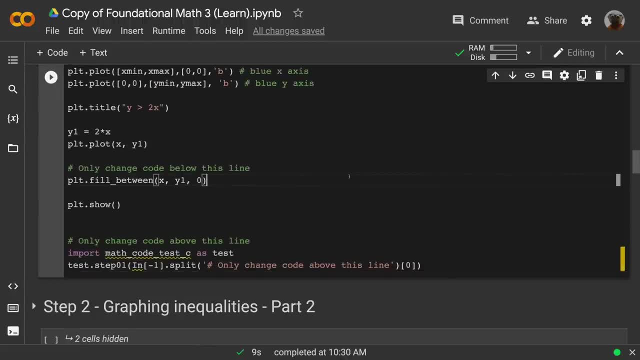 Then We Have The Second Arguments Are The Fill Between. So This One Notice We Have Here, You See, It's Fill Between, So We Still. 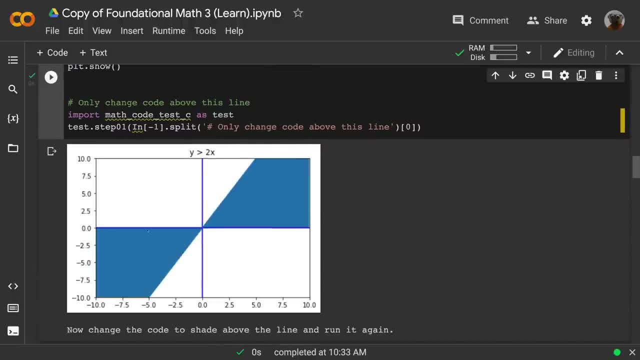 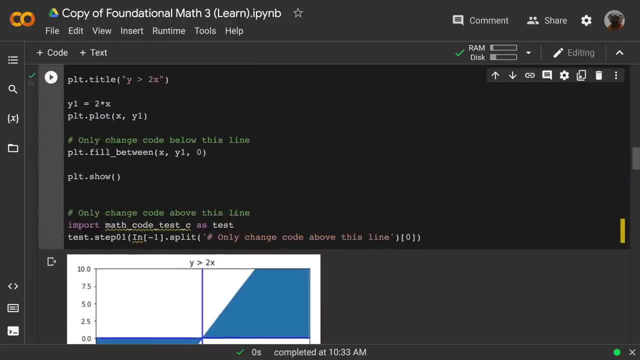 You See, It Fills Between- Why One And Zero, So That Doesn't Matter. You Know, That's Not A Consistent. You Know, Over On The 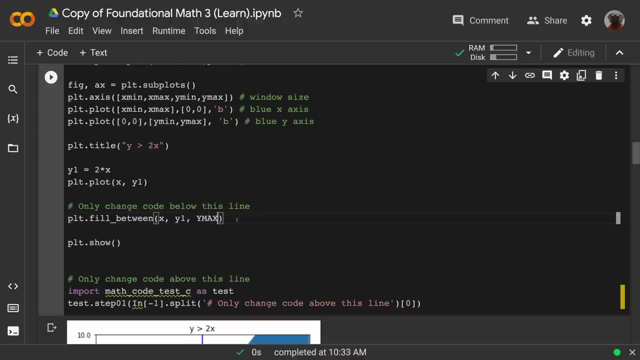 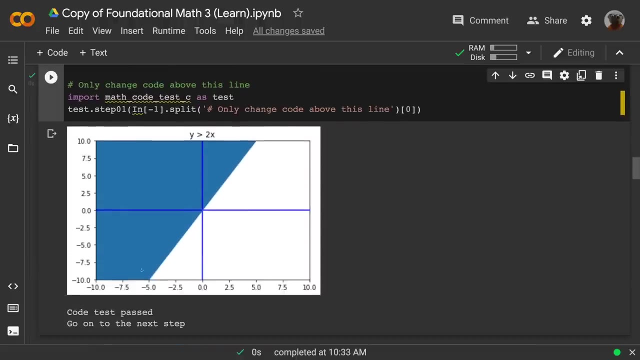 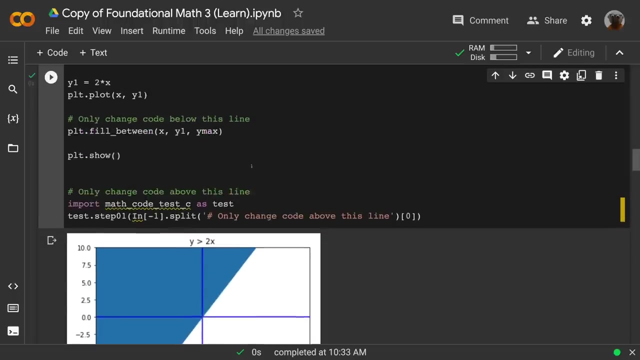 Left Here, Zero Is Up Top Without The Caps, And Then We're Always Shading Above Between That Line And The Maximum Y Value. So You 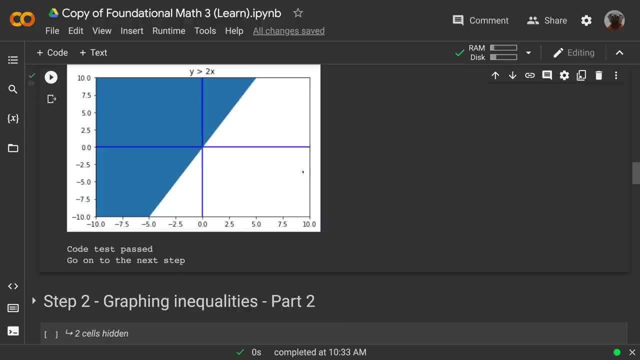 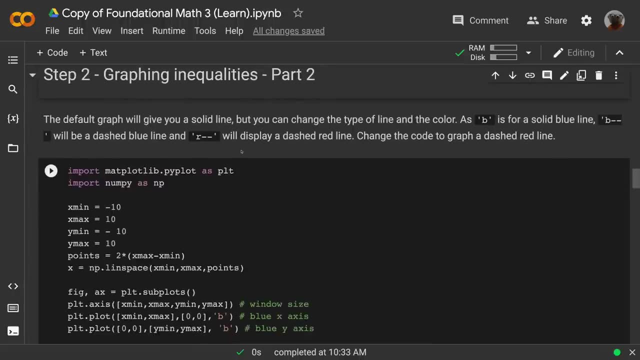 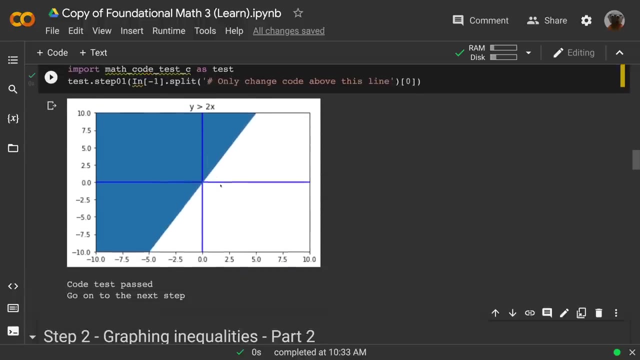 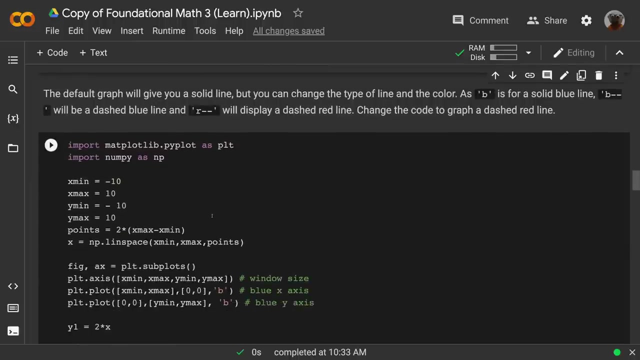 See Then Shade Below, You Can Change It To Y Min. Well, We Had This One Is A Nice, Solid Line And Remember Then That's. 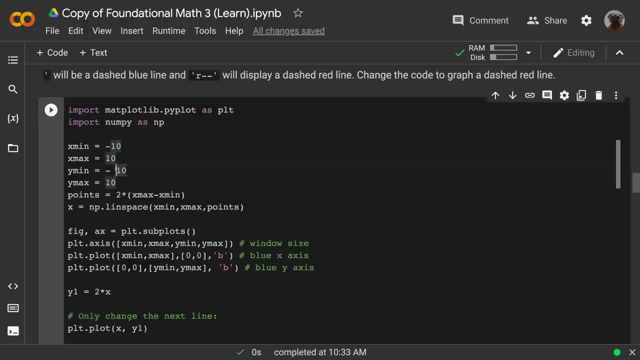 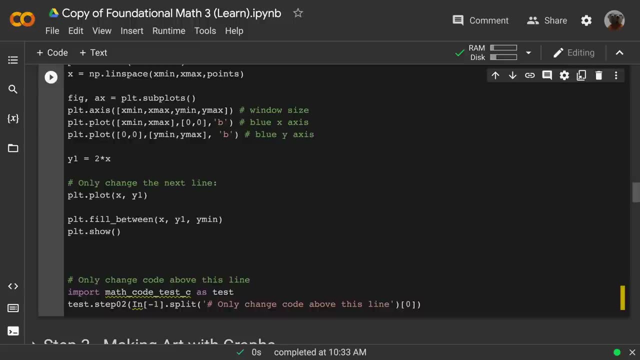 Greater Than Or Equal To. But What If I Wanted? You Know, Not That Solid. So, And This Is The Only Thing We're Going To. 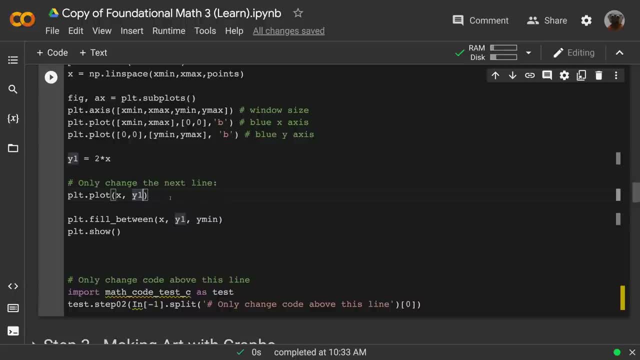 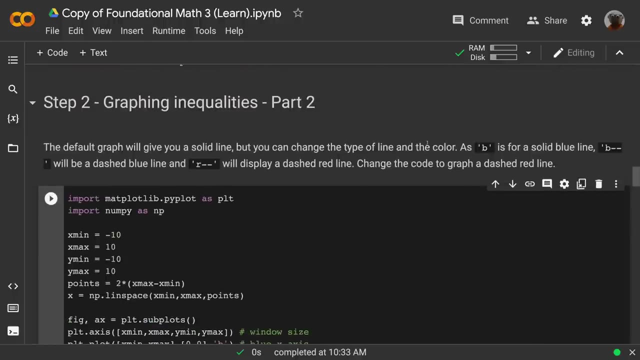 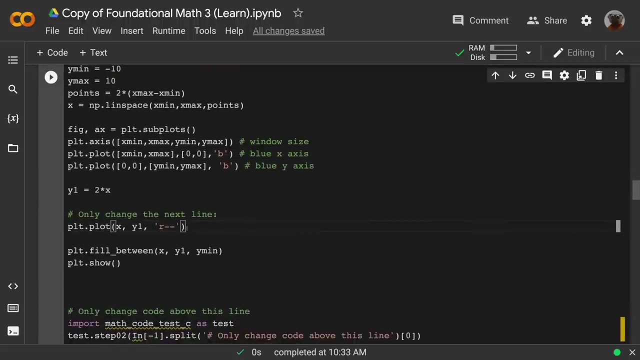 Change. If I Have This, Remember The Default Gives Me A Line Until I Do The Fill Between. But Dash Dash Um R. Dash Dash Gives. 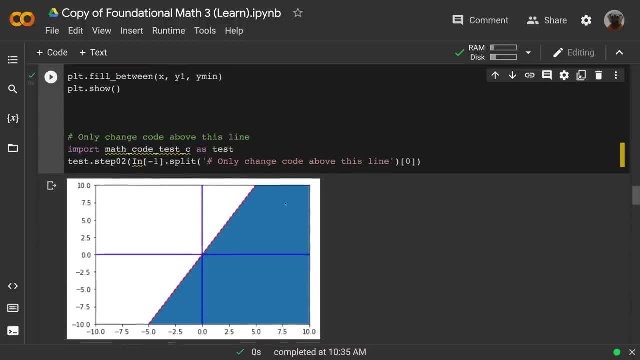 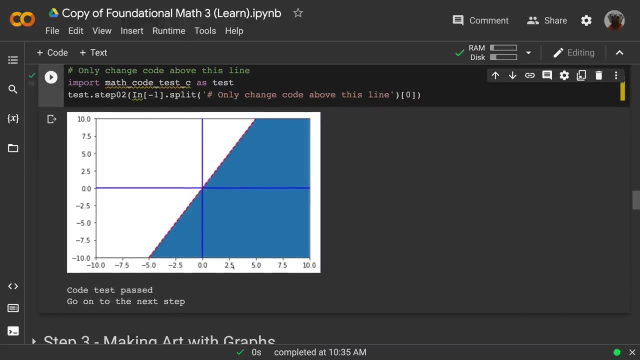 It A Dotted Red Line And We Run This. So Now We See, And Sometimes I'll Do That- I'll Make The Line We Can. 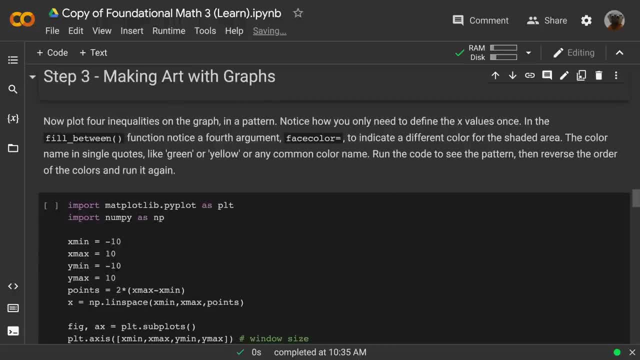 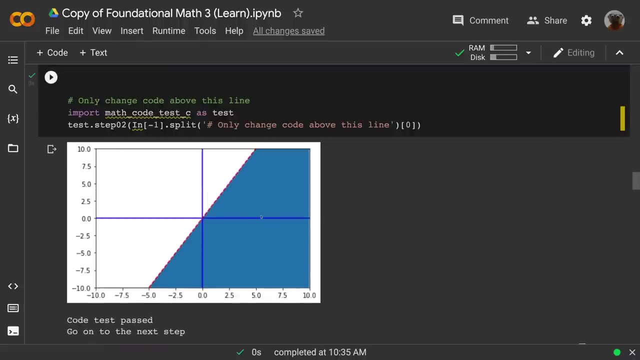 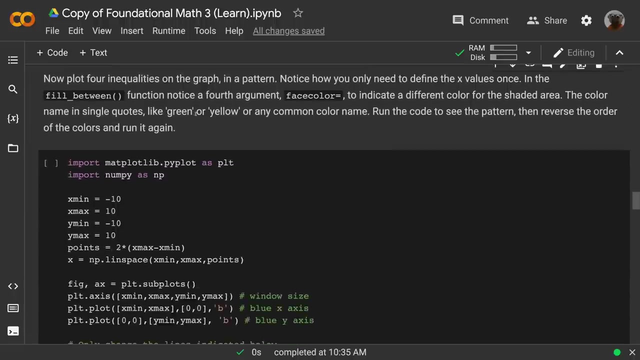 Make Some Lines. You Can Define These Lines, We Can Make Art, For Example. We Can Do That Fill Between And We Can Fill Between Two. 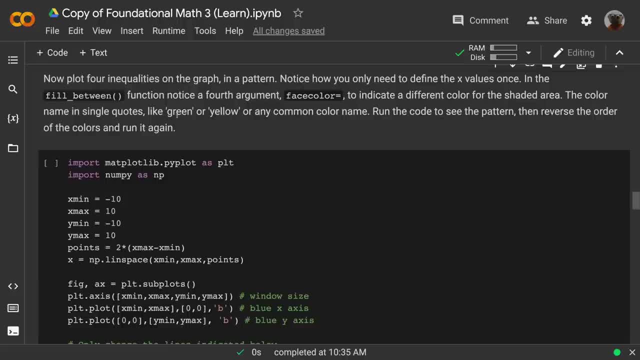 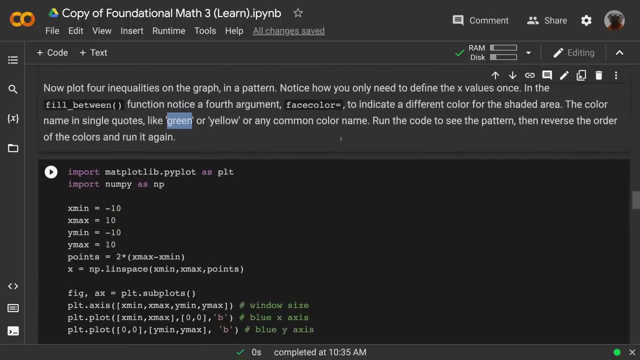 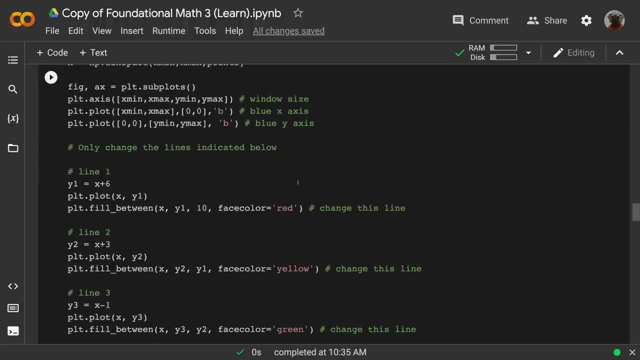 Different Lines If, Like A Lot Of Your Basic Colors, You Actually Can Just Get Away With Just Putting That. You Know I Want To Be. 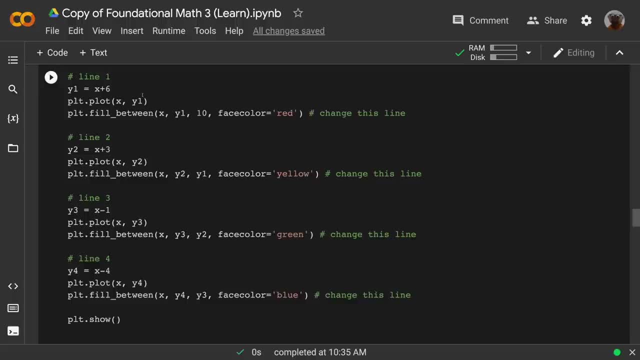 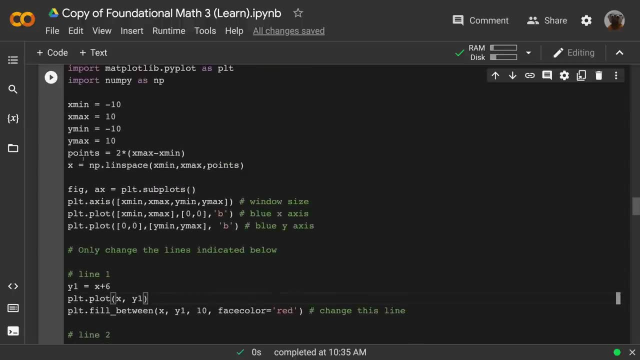 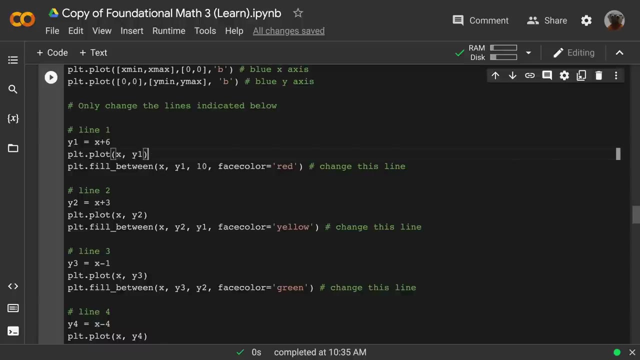 Green. Putting Green In The Graph Is The Line We're Plotting, And Remember We Defined The X Value Up Here Once, So Here's This. 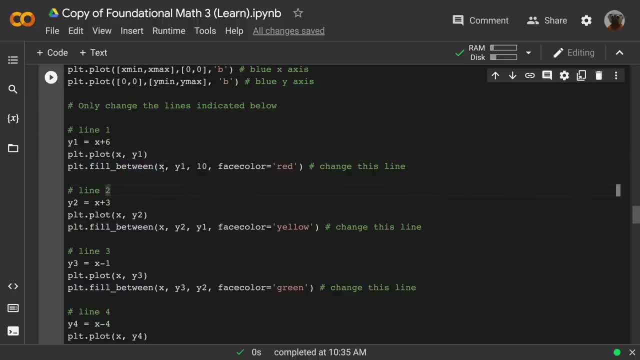 Y Value. Plot This. I'm Not Worried About Making A, Make It. You Know Why, Max, But That's Fine. And Then I Had The 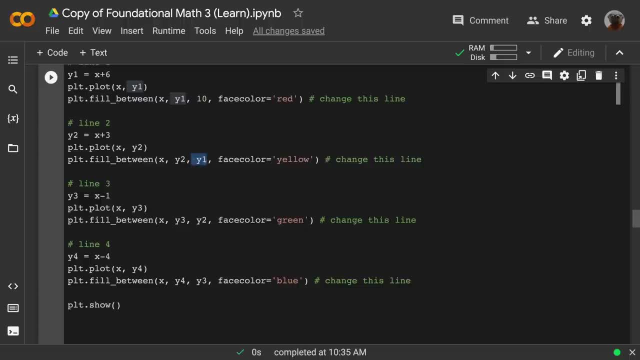 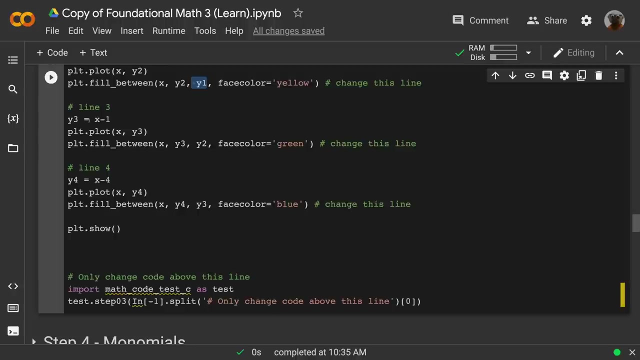 Other Argument: Face Color Red Line Two: I Have This And Fill Between. Now Notice Between Y, 3. So Then Change This. You Know We. 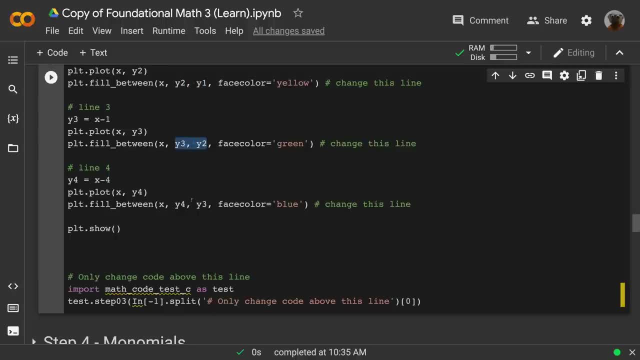 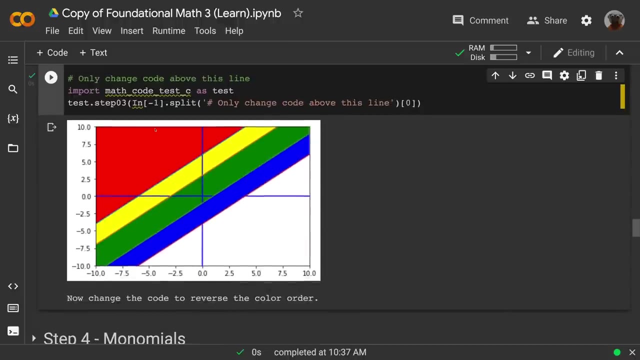 Have This Color And Same Thing, All These. You Know This Line Y, 3. And I'm Going To Fill Between These Colors. So If We 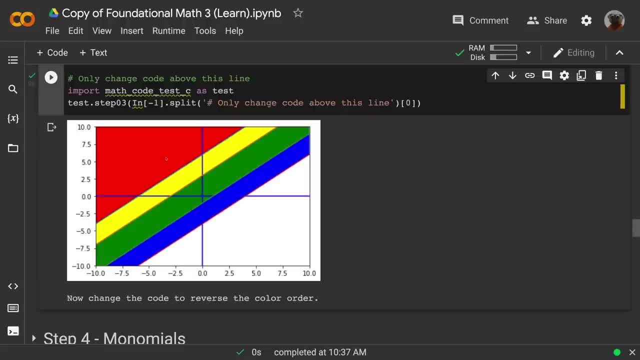 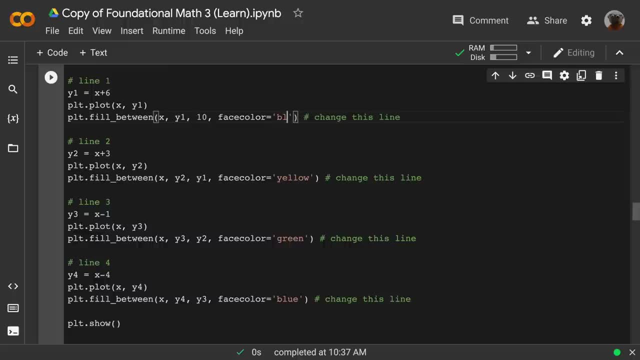 Decide To Have Another One To Fill Down To The Bottom We Just Left Here. So If We Take This And Reverse The Colors And The 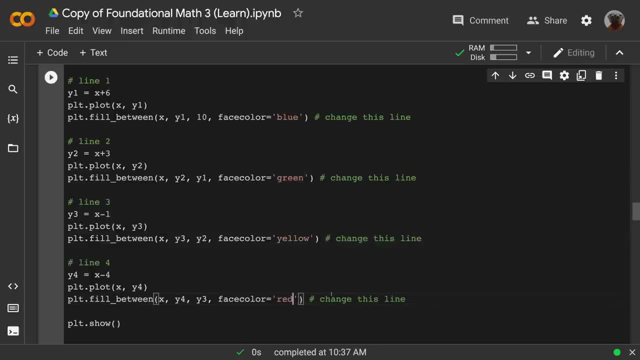 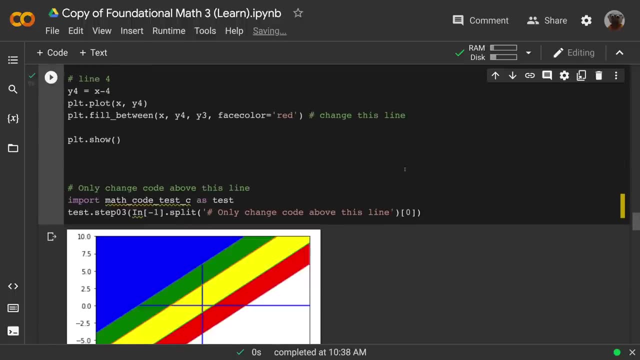 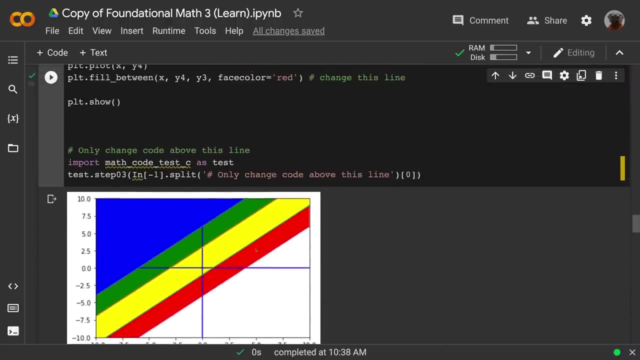 Next One Will Be Red. There We Go. So Now We Have This And We See When We Run It Reverse The Colors. So There We. 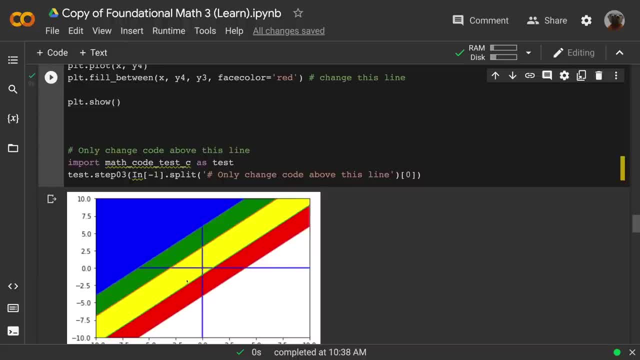 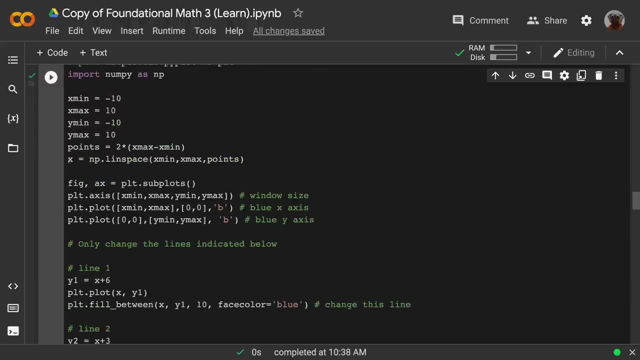 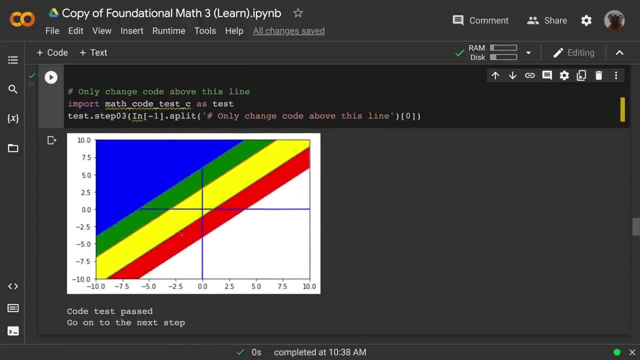 Go To The Bottom. We Have One, We Have The Colors And We Go To The Bottom. We Go To The Colors And We Go To. 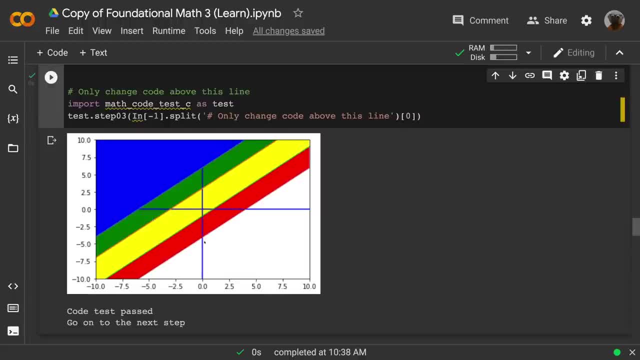 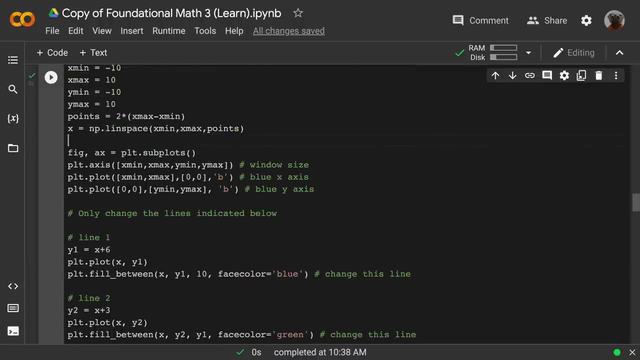 The Bottom. We Have Within Certain Values And You Can Make All Kinds Of Shapes And Then Continuing On What We Were Doing With Other. 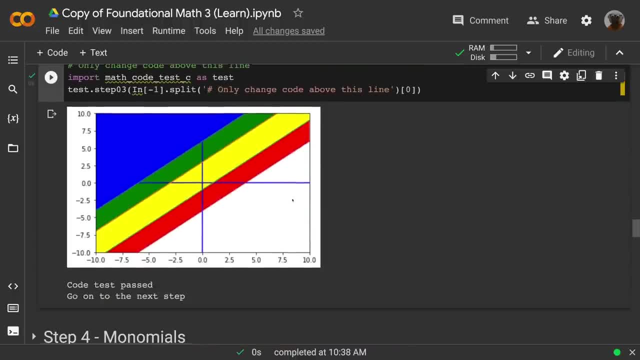 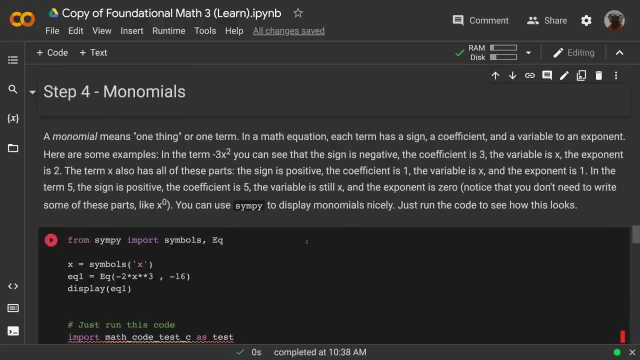 Graphing, I Kept These Axis Lines, But You Can Make All Colors. And Now We Get Into Looking Further, Into Factoring, Into Representing Equations. 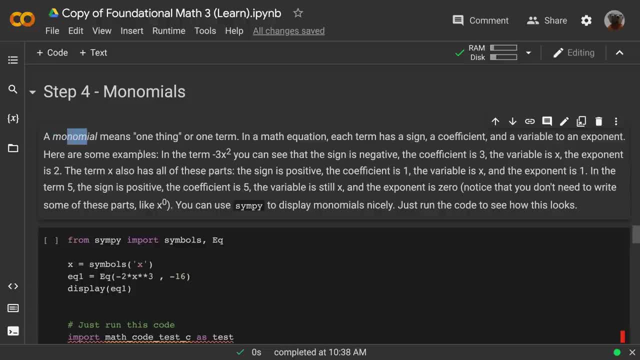 So Monomial Is One Thing, We See That Mono Is One, And Then It Has A Sign: Coefficient And Variable And Exponent: We Don't. 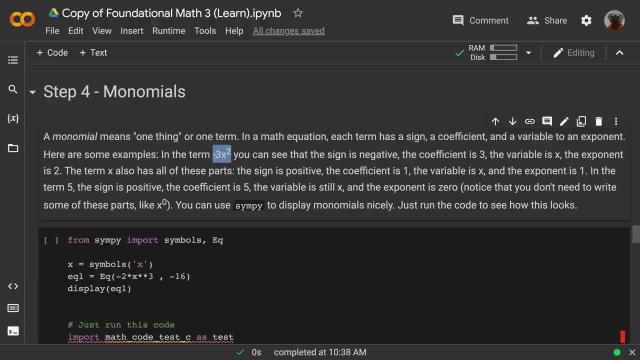 Think About That All The Time, But When We See It Here Definitely, I See A Negative Sign. I This Is Positive. One X To The 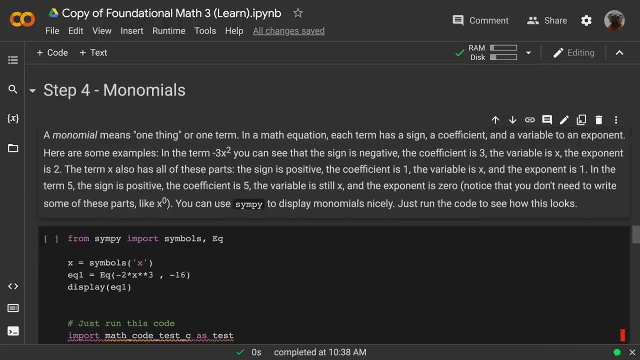 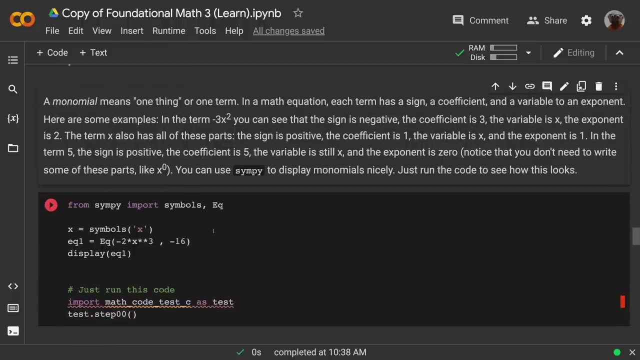 First Power. Just Things To Think About, Because That Really Comes Into Play For Some Other Things That We Do With Factoring And Just Make. 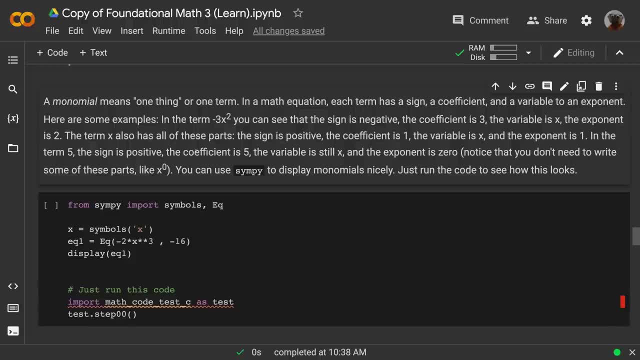 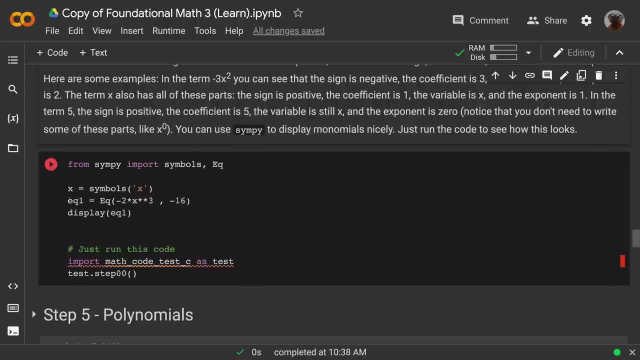 Sure That You Define Each Of These, Even Though Sometimes These Values Might Be One Or Zero And You Might Not Display Them. So Here We. 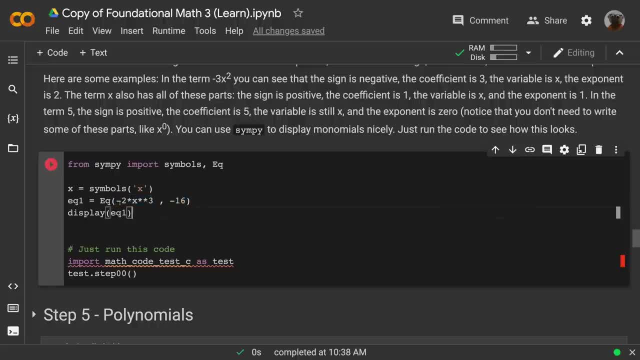 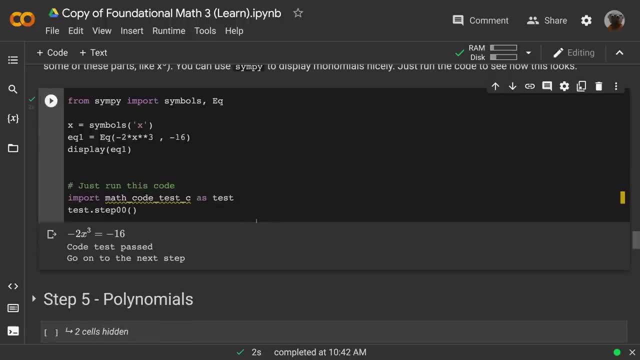 Define What Is On The Right, So I Define It As An Equation, And Left And Right Just Get Separated By A Comma, So You 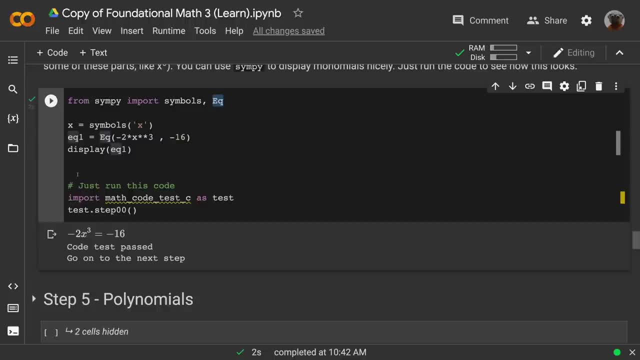 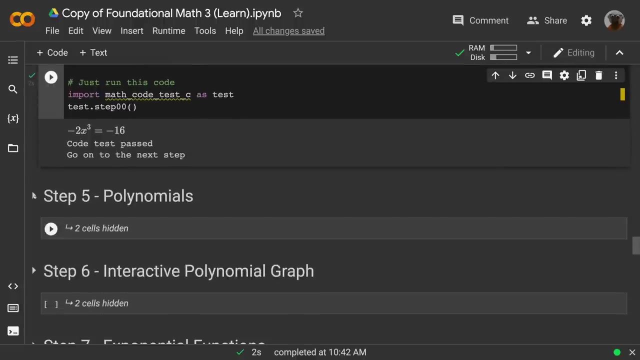 See What We Have, And You Know, Bring Up E, Q. You Know, Use Your Variables That You Already Have. And You See, We Just Define. 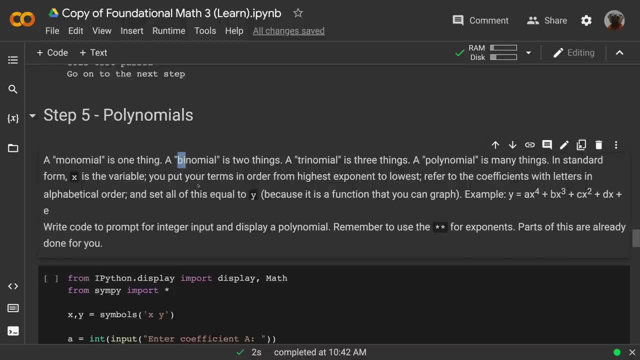 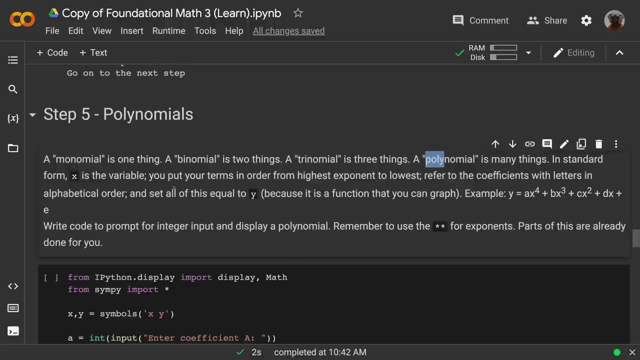 X As The Symbol Here, So We Have Three, And After That We Kind Of Stop Counting. So Polynomial Is Just Many, Poly Is Many. 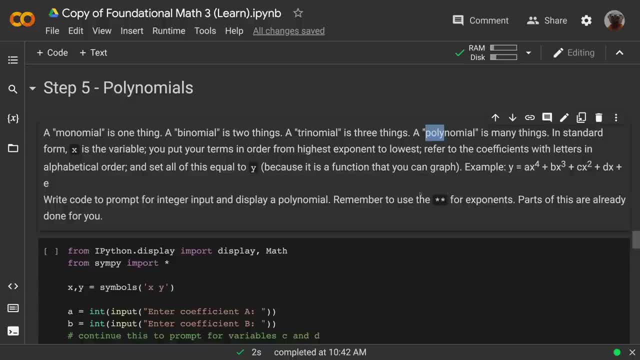 And We Usually Put Them In Order. So We Take X. What I Can Do Is, If I Know, This, I Can. This Is The Normal. 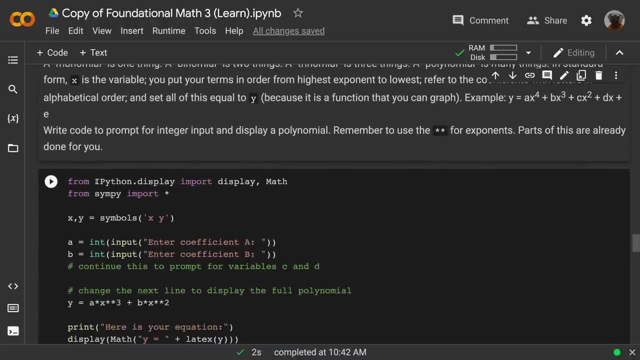 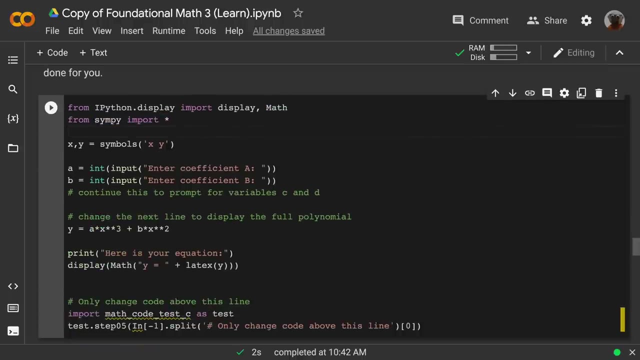 Standard Standard Form Setup, So You Could Prompt For Each Of These Coefficients And Import Everything From Simpi. So Now We Have These Symbols. 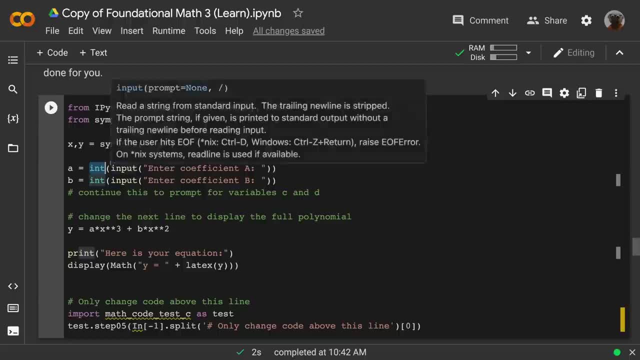 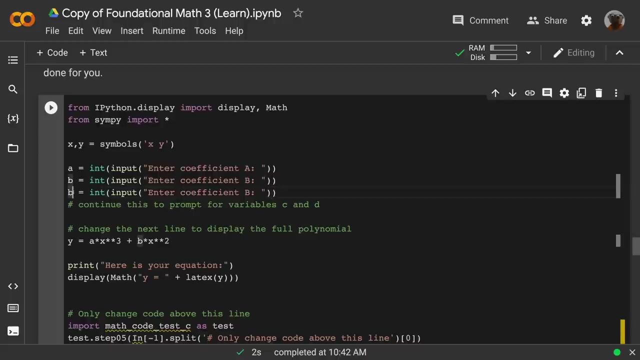 And We Want A Coefficient. And, Yes, I Do Want To Cast As An Integer, Though I Mean Realistically And Make This See Input Coefficient. 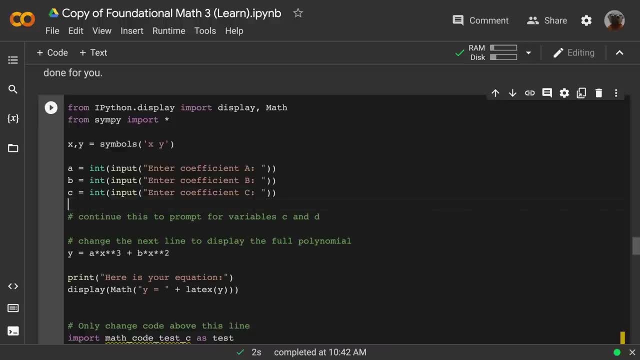 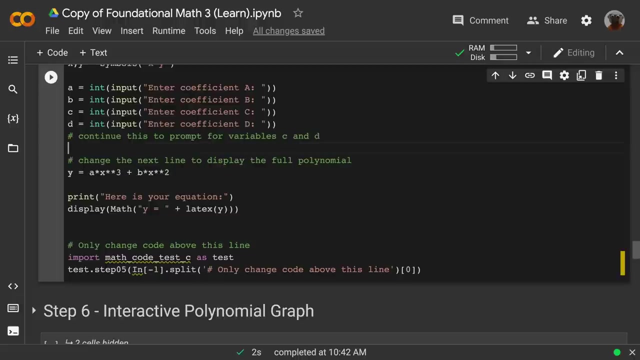 See, And Then Will Do For D Input Coefficient D. All Right, So Now We Want To Display The Full One, So We Have, We're. 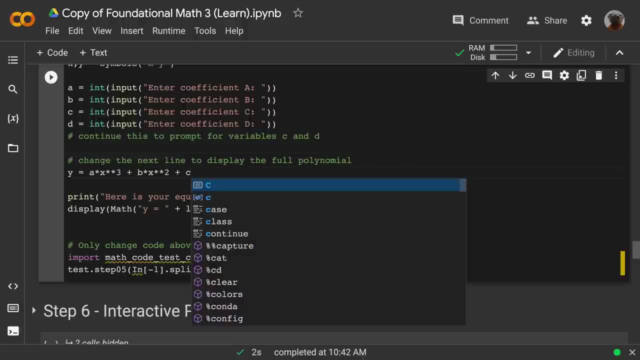 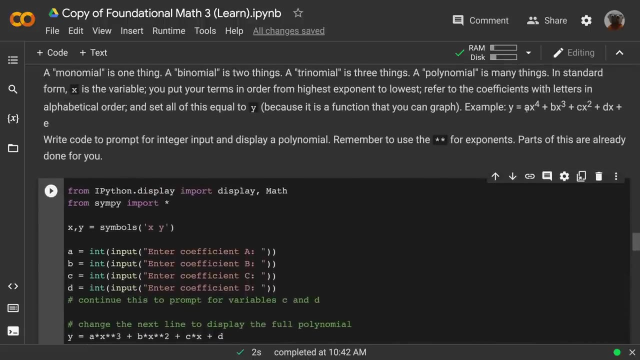 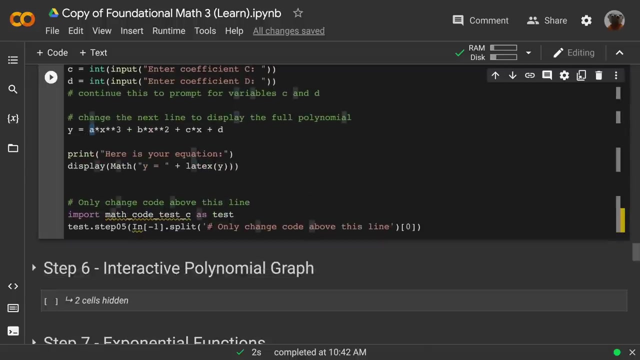 Going To Display A X To The Third, B X Squared, And Then We Do The Rest. I Just Put These Right Next To Each. 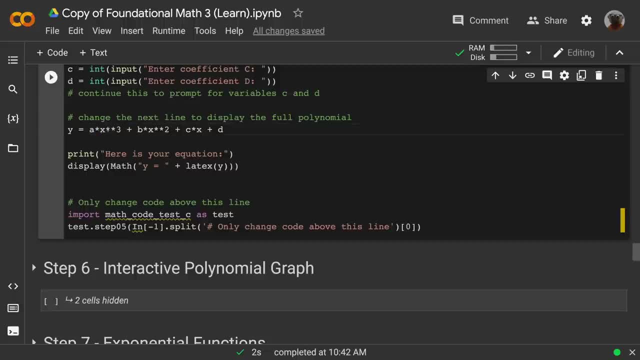 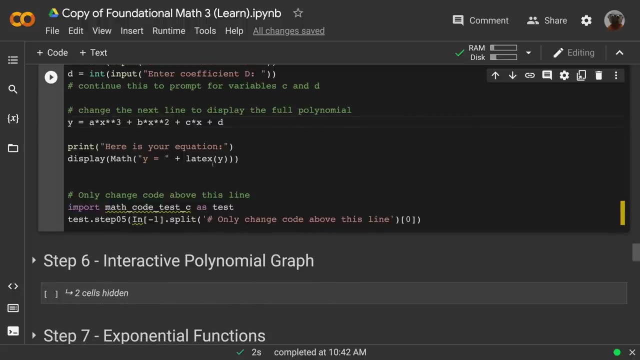 Other, A X Means A Multiplying, But Remember The Python Notation, I Have To Put That Multiplying In There, So It, Oh Well, I. 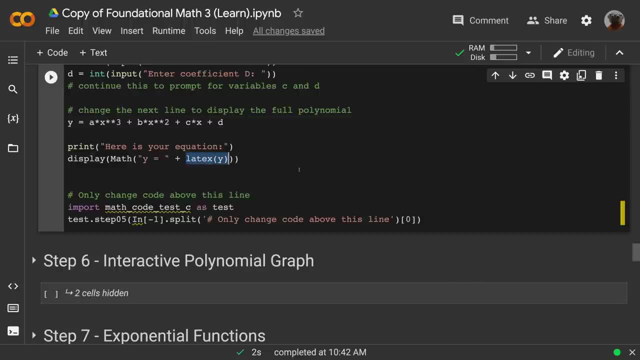 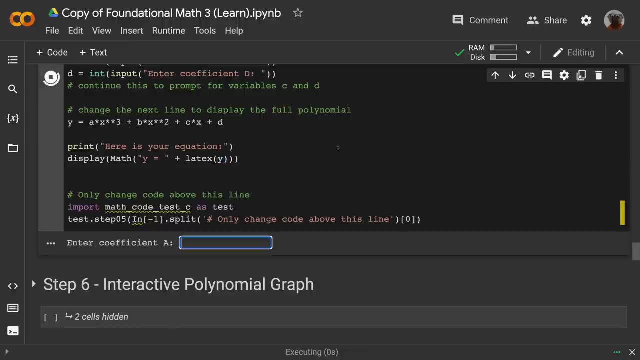 Have To Convert That To Latex, Which Is Really The Way We're Going To Display Math, Terminal Math Formulas. So Now We Have This: 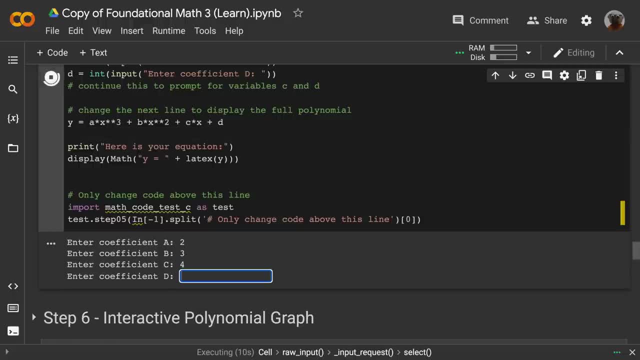 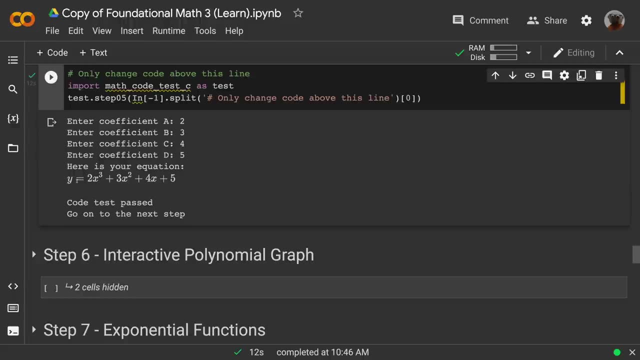 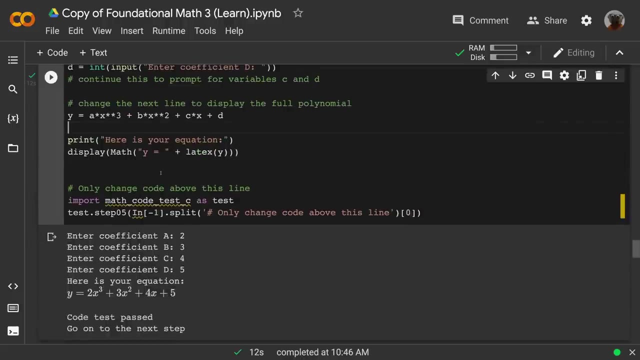 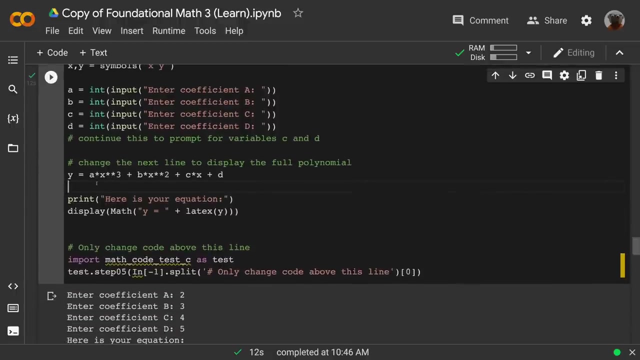 I'm Going To To Convert This, To Convert This, To Convert This, To Convert. That Way, You Have All This For Things You Know We're. 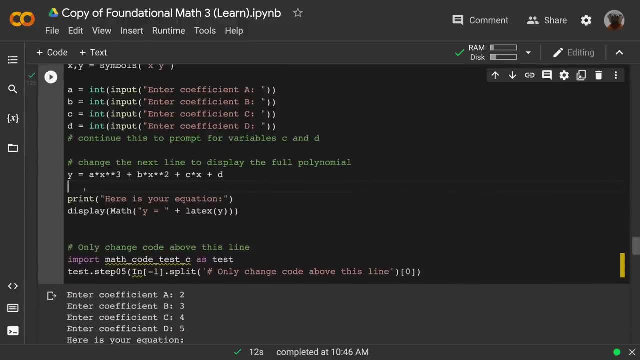 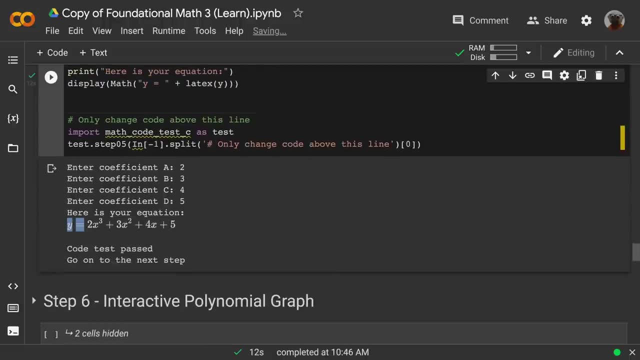 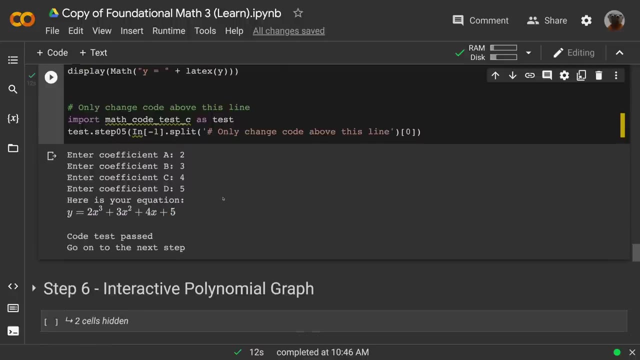 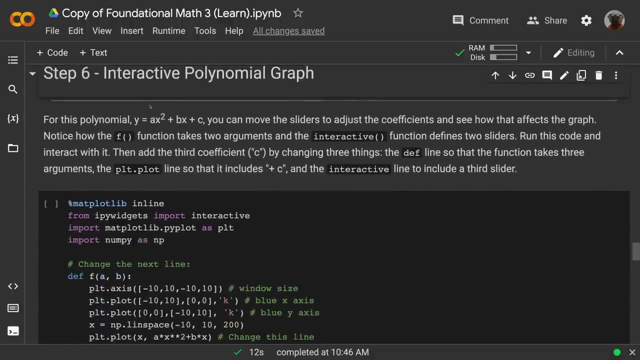 Thinking Ahead, We're Building Things That Display This, This Formula, In A Nice Way. So There We Go. That's What We Have And, Yes, That. 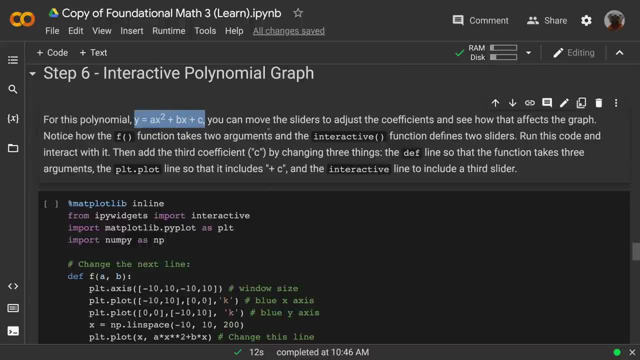 Does Look Nice. So This Is Going Through, We're Going To Adjust Each Of These Coefficients. So, Again, In Doing This, This Certification Notebook. 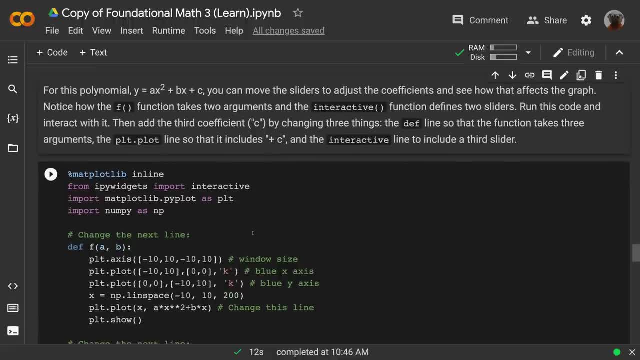 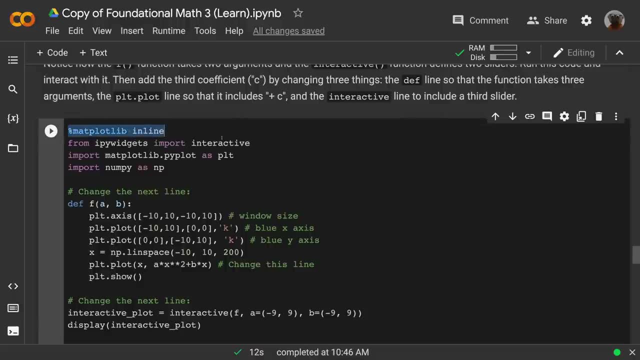 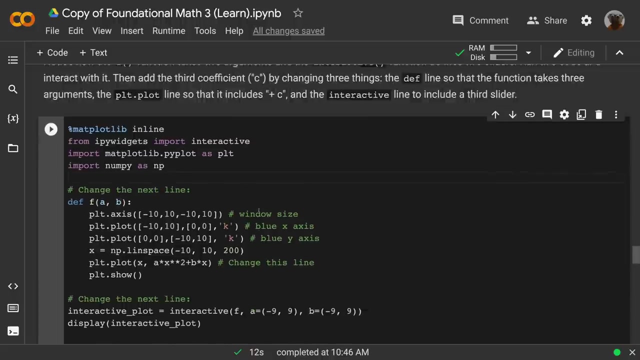 You Should See. This Is Coming Up. You Know Things That You've Done, Bring In Interactive From The Widgets. There We Go, All These Things. 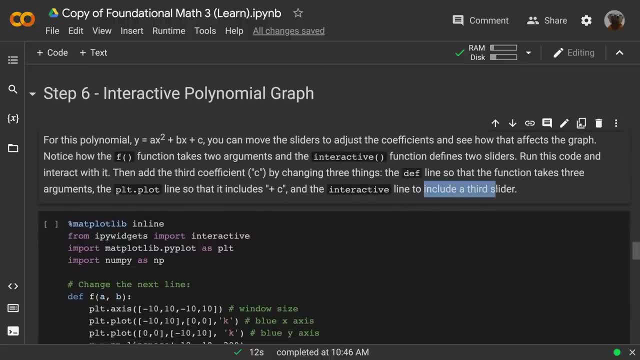 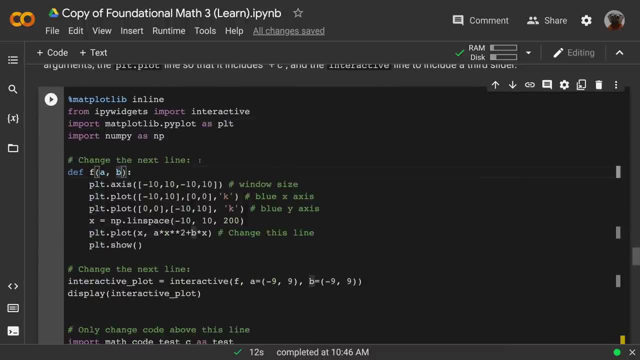 And Remember These, The Function Of A, B, And So For This One We're Going To Change To Three Inputs, Great, And Then All The 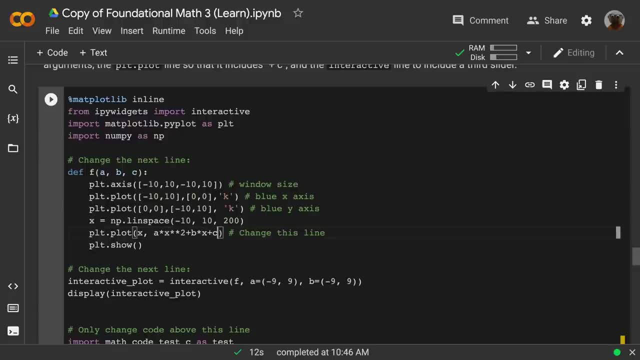 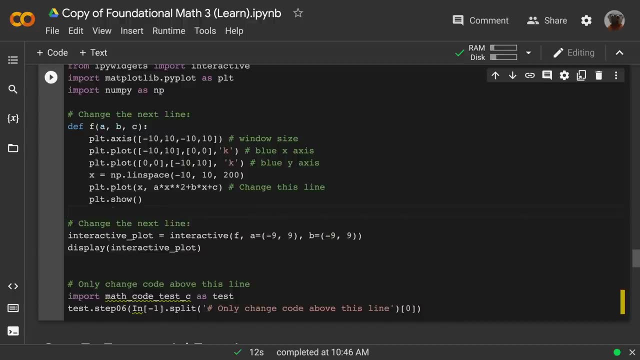 Rest Of These Are Fine: A X Squared Plus B X- I Have To Add This Plus C, And So That Will Show We Can. 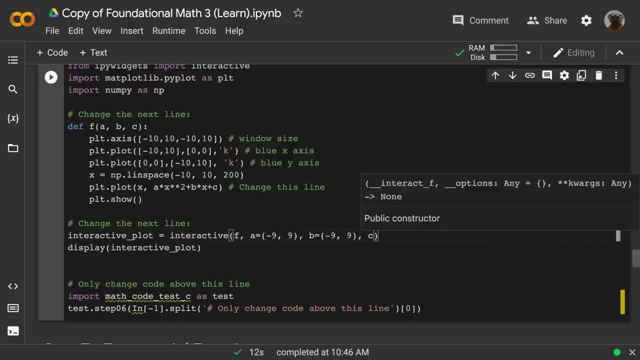 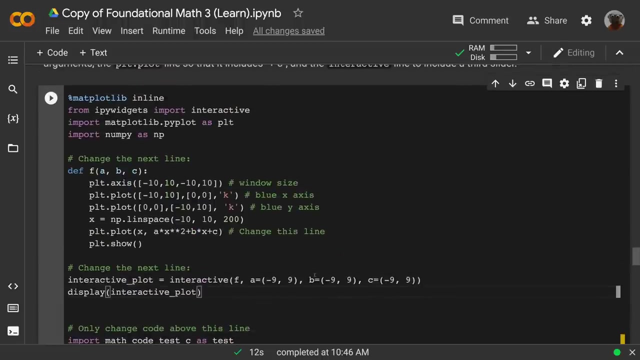 Just Copy That Comma C. So Now We Will Have Three Sliders: A, B And C, And We Have The Interactive And Then We're 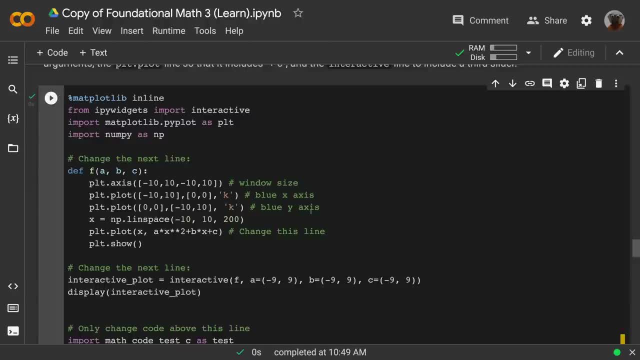 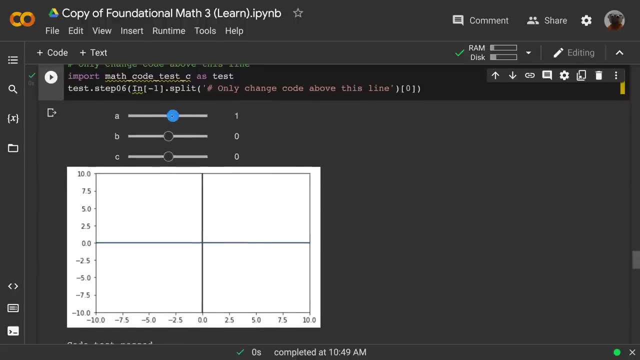 Going To Have Four Coefficients. So Now We See, And Looks Like Nothing, Because Everything Is Zeroed Out, But As Soon As A Gets. 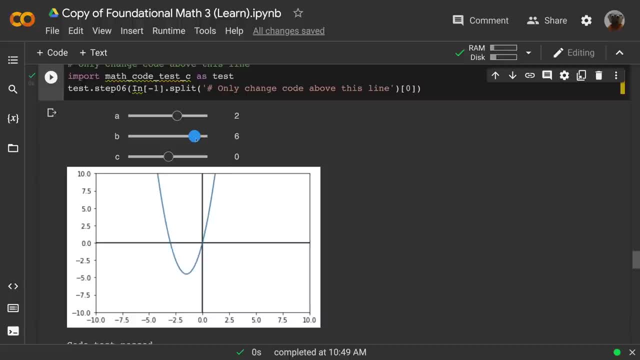 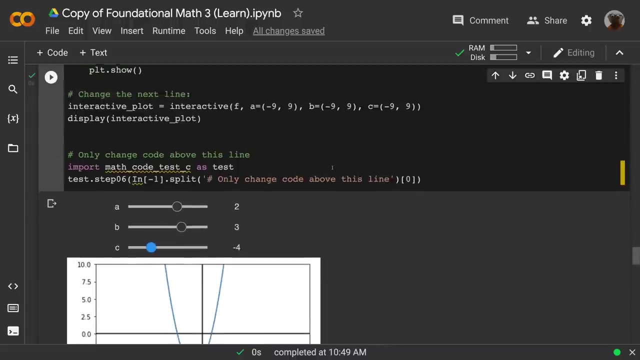 To Be Something Then We Have. So You Can Tinker With This And See, Remember That Just Moves It Up Or Down. There We Go. 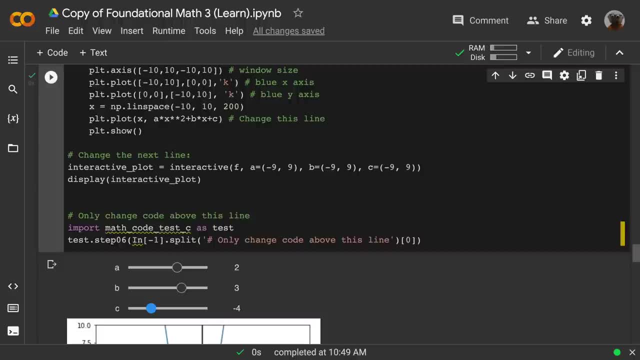 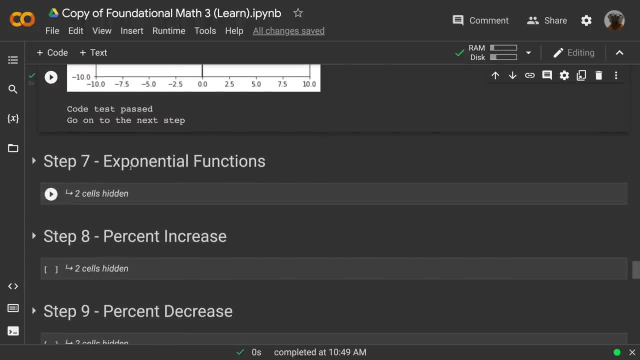 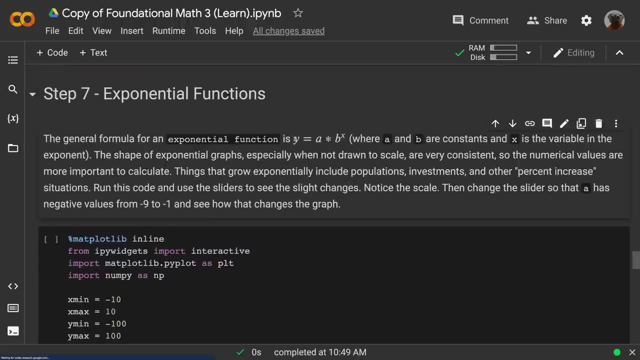 So You Can Take These And You Can Tinker With These Sliders And See What Looks Like. So Now We're Going To Exponential Functions. 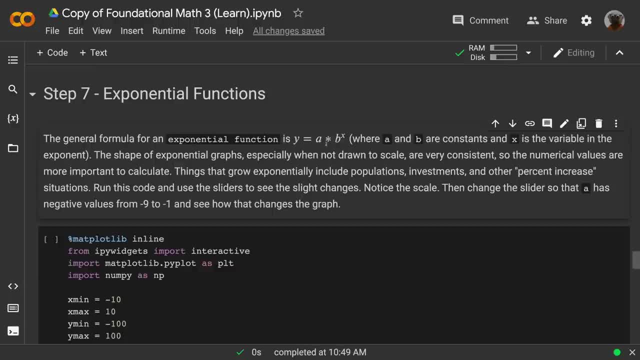 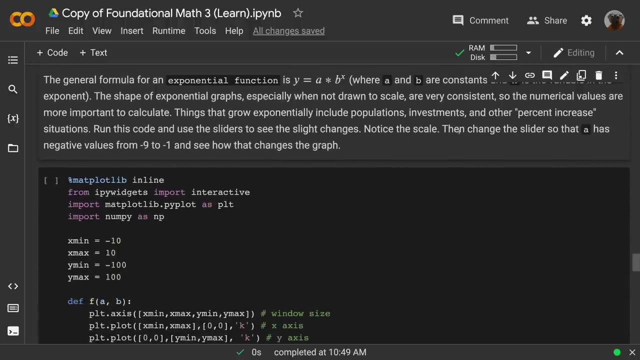 And Remember Our Exponential Function: Y Equals A Times B To The X. And There We Have All Right. So Again, Thinking About Some Of 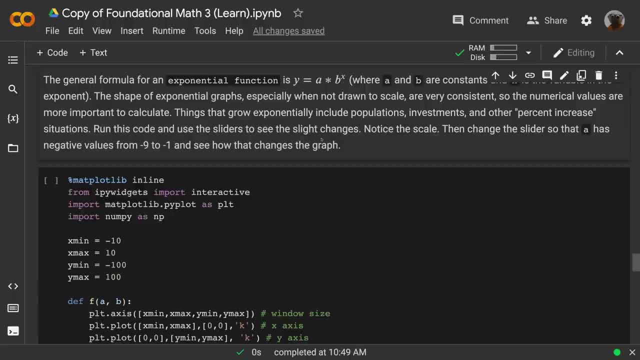 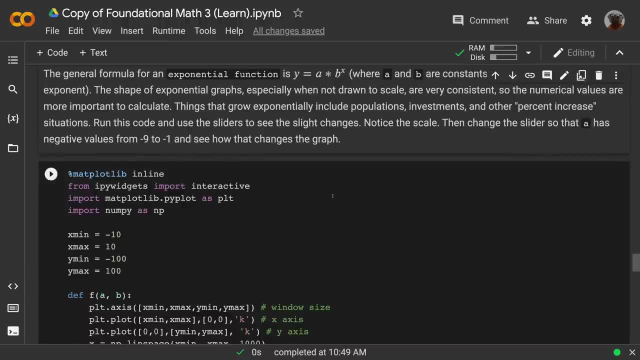 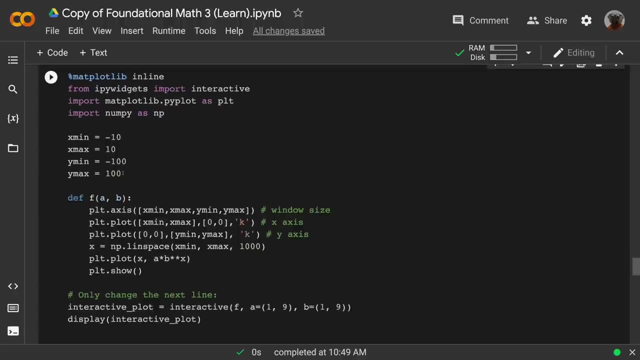 The Exponential Functions, The. So What We're Going To Is We're Going To Run This Code- See The Sliders- And Y Maximum- A Lot. 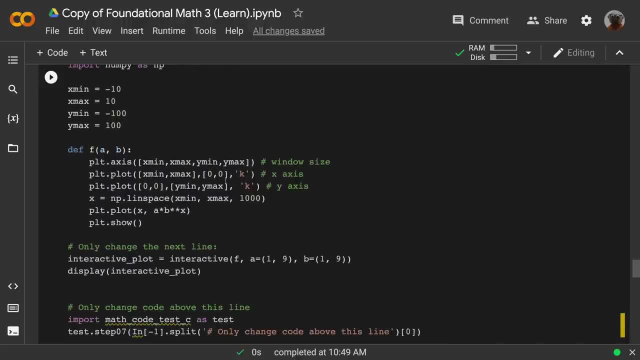 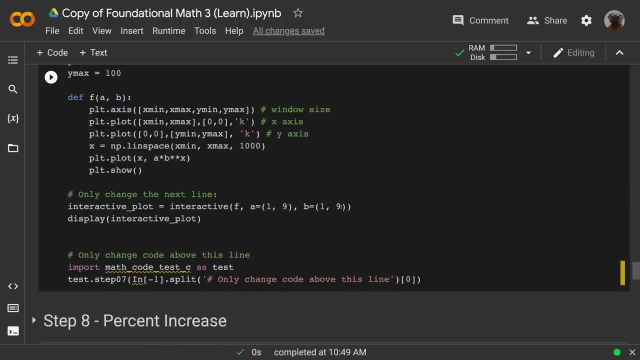 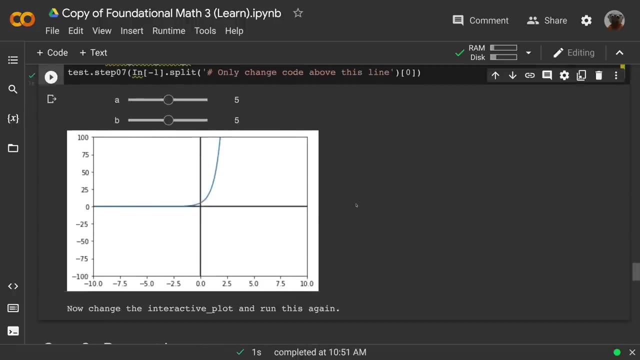 Bigger Things Grow Exponentially, So Kind Of Need This To Display A Decent Graph Here. We Just Have A And B And You See. 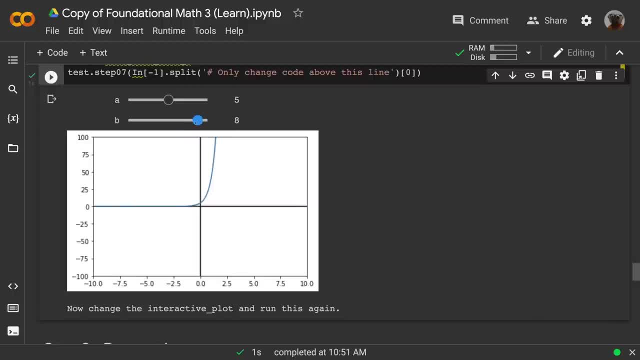 One See, As I Increase This, It Gets To Be Steeper. But We See The General Shape Of This: It Just Gets To Be Steeper. 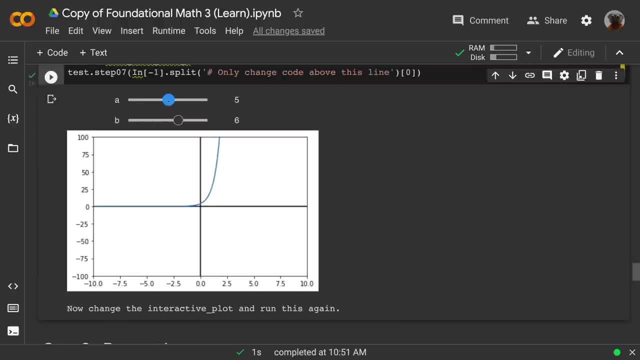 And Then If I Change A, Do The Same Thing. Maybe B Has A Little More Of An Effect. But Then You See, It's Kind. 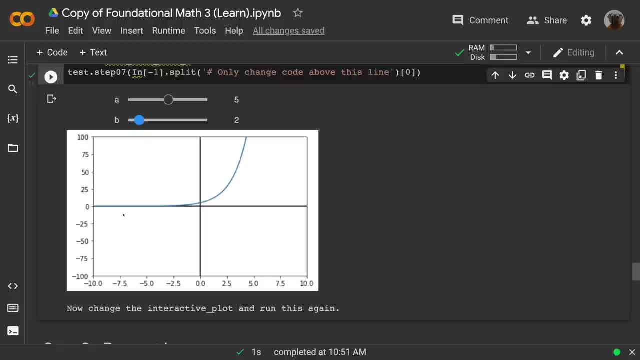 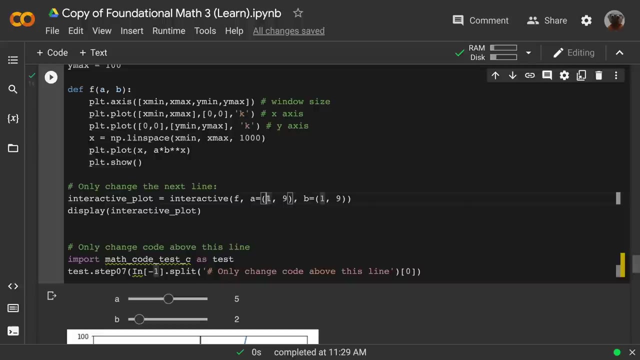 Of That Same Upwards, Upward Curve, And Then As The And Then Looks Like It Does. But If You Zoom In, Doesn't So You? 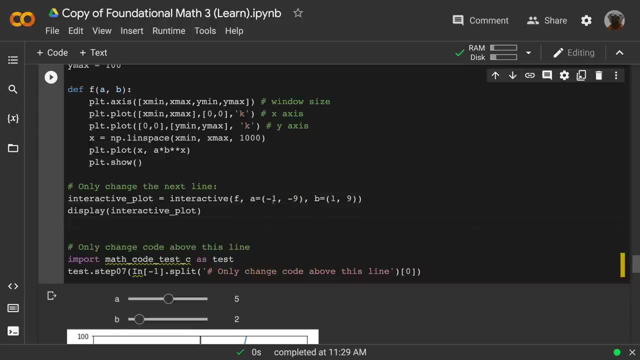 Know That's The General Trend. So If We Make This Negative, Then We Still Need The Low Value, And Negative One Is The High Value. 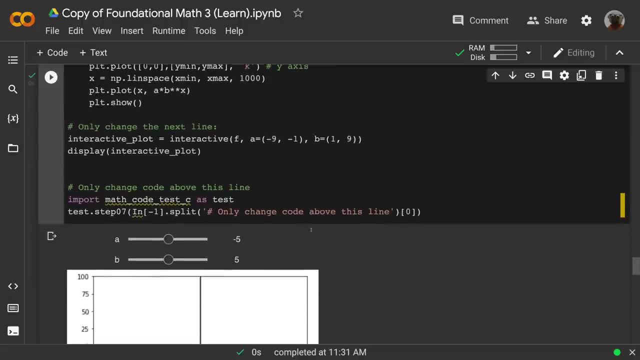 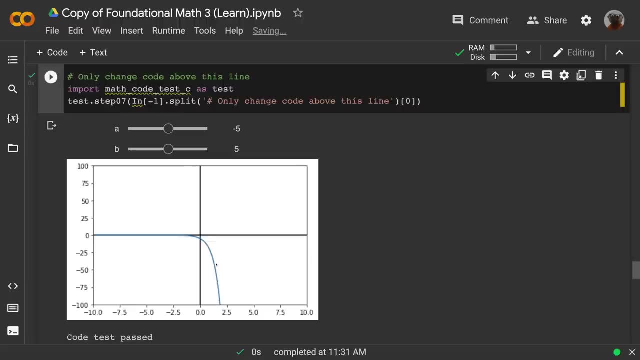 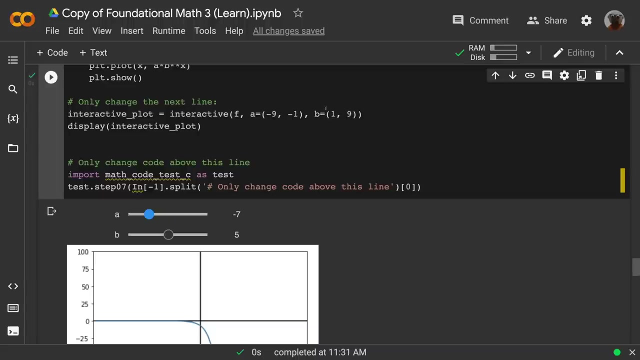 Remember, Because It's More Negative. So If We Don't Switch Those Also, Then We Would Get An Error. So If We Make This Negative, I'm 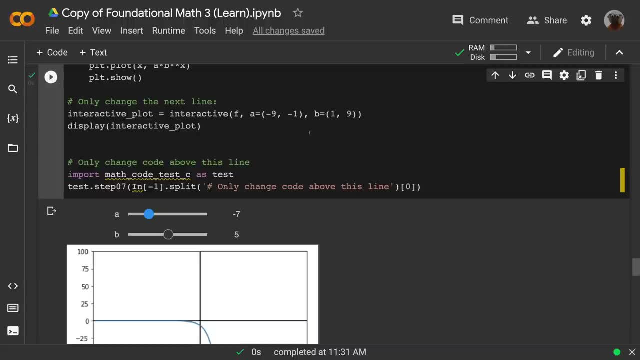 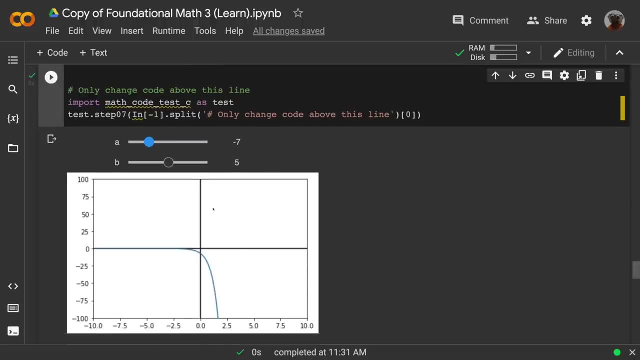 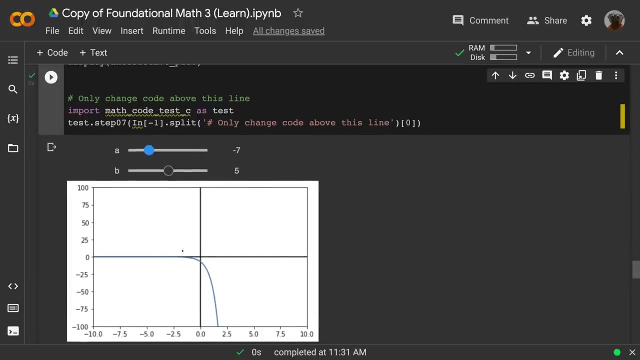 Not Going To Even Worry About Doing This Right Now, But If We Did That, It Works For Integer Values Of The Exponent Be Mathematically. 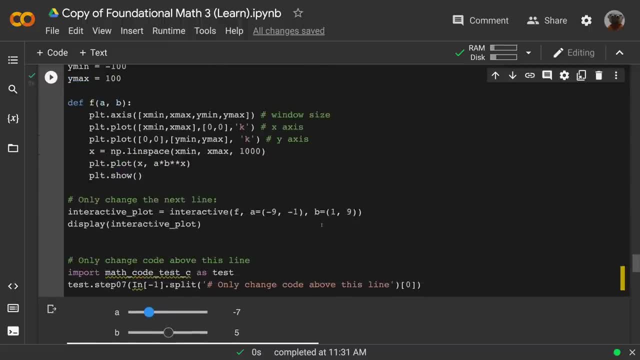 Doable. Also In This Case They Would Actually Be Imaginary. They Wouldn't. They Would Not Necessarily Work Out Well Sometimes If We Had You. 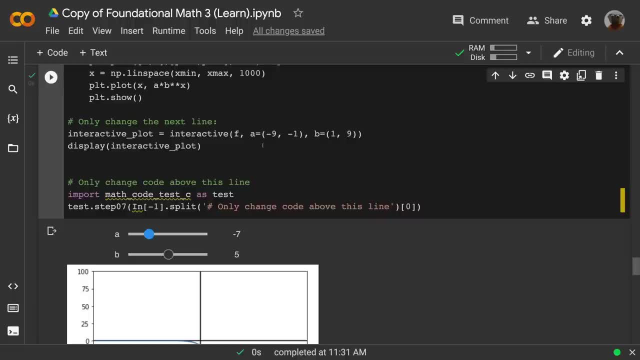 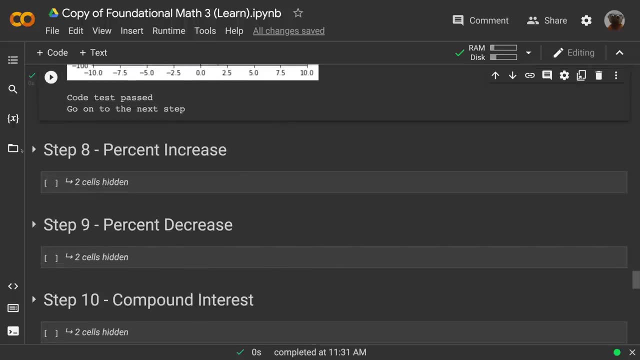 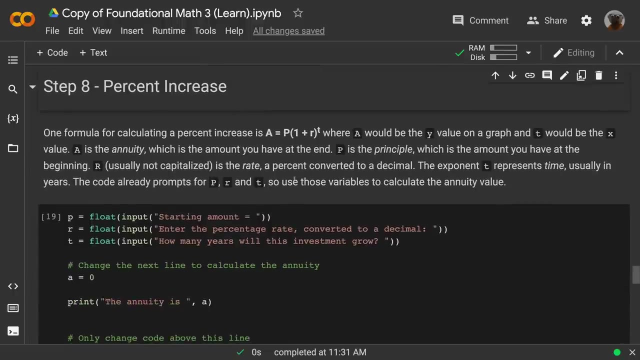 Know Some Of Some Values But Doesn't Work Out Nicely For Others. And A Graph Would Be A Mess. But Let's Look At Stuff. 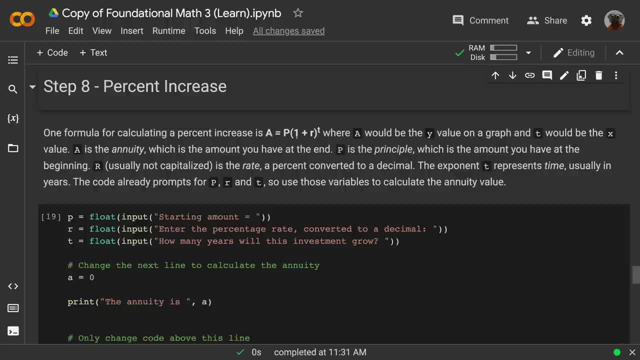 That Does Work Out Nicely: Percent Increase. So I Value If You Were Graphing This And You Would Know P And You Would Know Our. 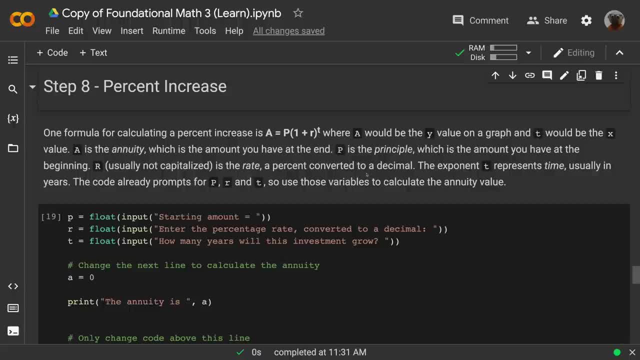 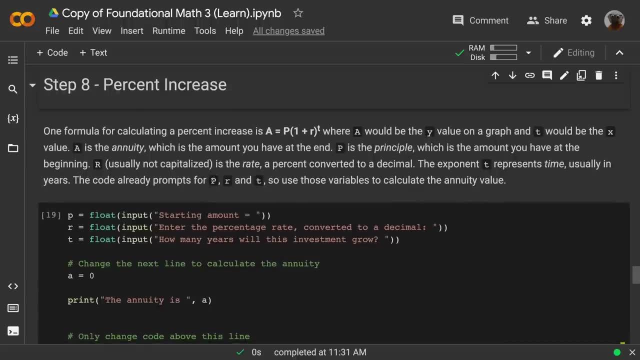 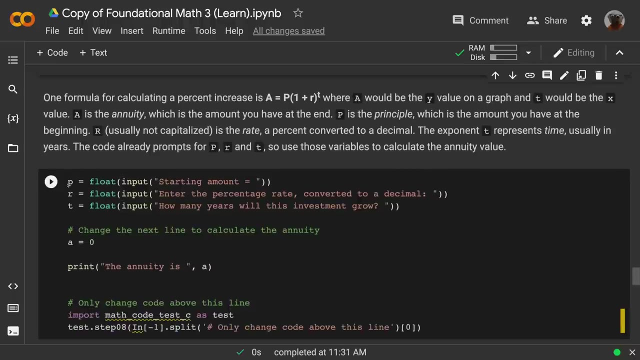 So T Would Be Time In Years. But That Would Be. The P Is Capitalized. So Just Interesting In My Variables I Kept Them All. 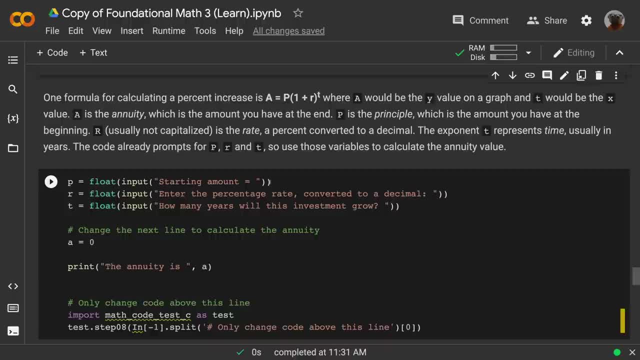 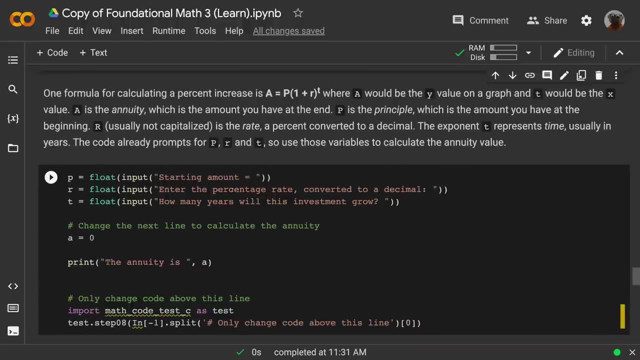 Lowercase, But A Lot Of Times You'll See That Written. You Know Their Lowercase But P Numbers, Percentage Rate Converted To Decimal And How. 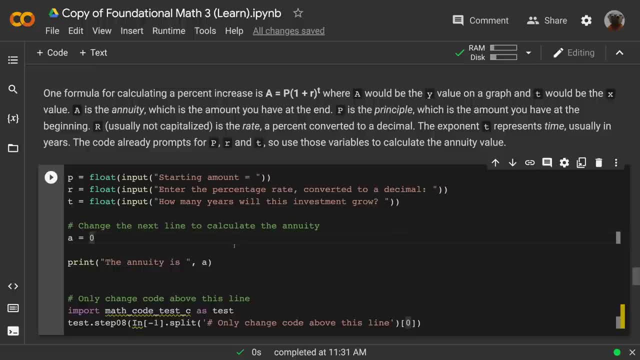 Many Years. So We're Just Going To Take This Equation And Put It Down Here In Python Terms. So We Have Of Time And There. 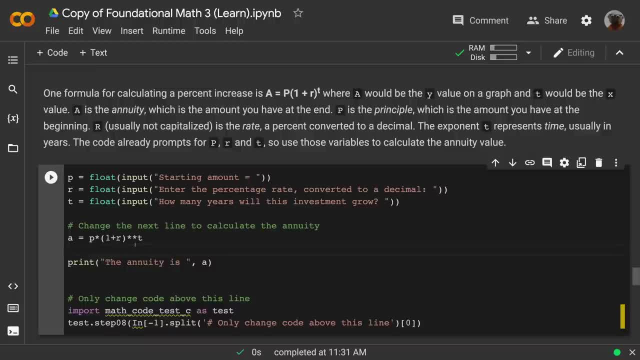 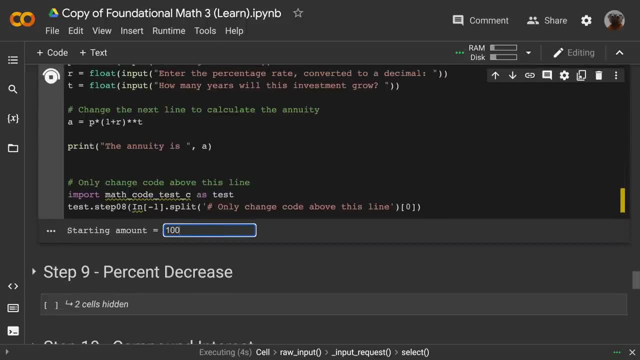 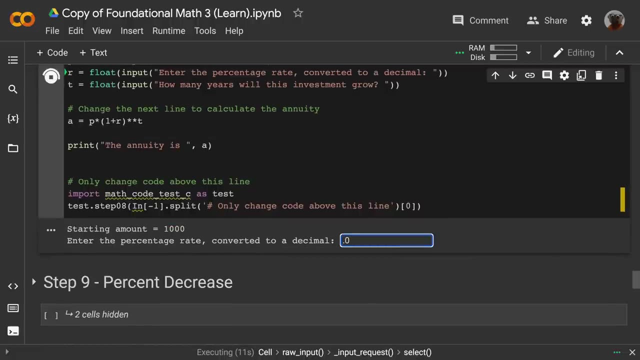 We Go Just Translating That Equation To Python And Then We'll Print Out The Annuity. So We Run It Starting About 1000.. 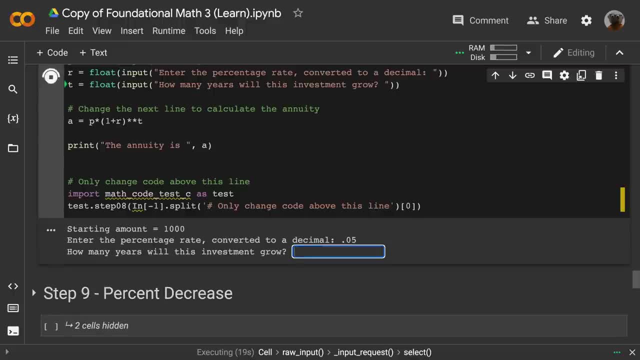 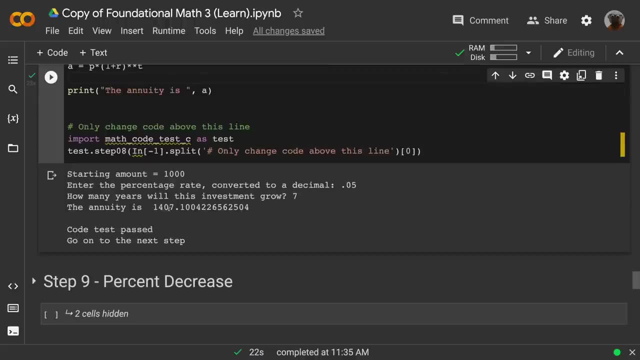 Just Take These Nice Let's Say Like Seven Years. All Right, And I Didn't Worry About Putting In Another Function Around This, But You 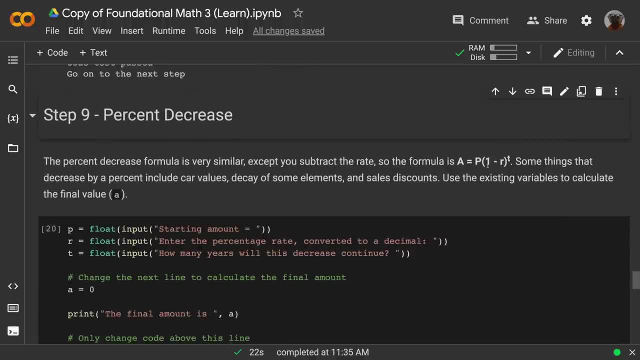 Probably Would, But There You Go To Two Decimal. That's The Rate And This Does, This Does Happen. We Have Car Value, Values Of Cars. 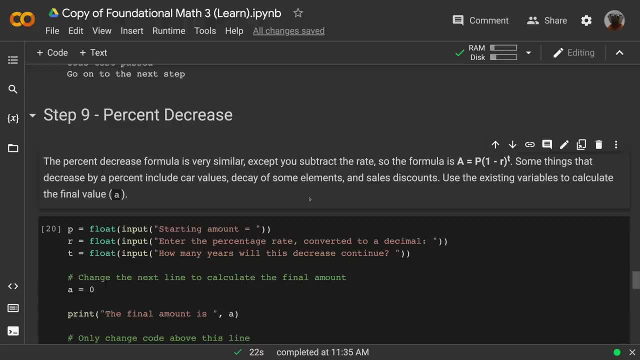 Or Some Other Products That Might Decrease At A Certain Percentage Rate. Every Week Of Something, Some Sales Discounts, Maybe There's Something That Decreases. 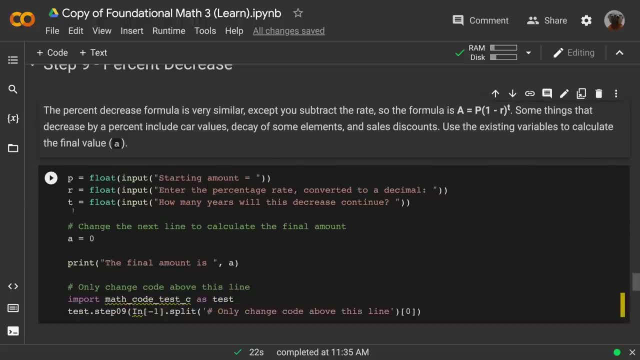 At A Percentage You Know, Every Week If It's Not Sold. So You Have Some Applications Of This And We See You Know The Jupiter. 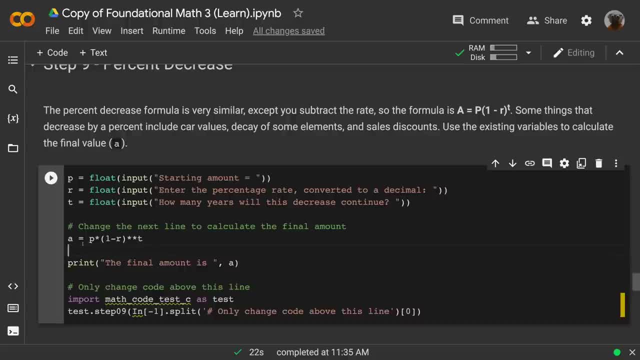 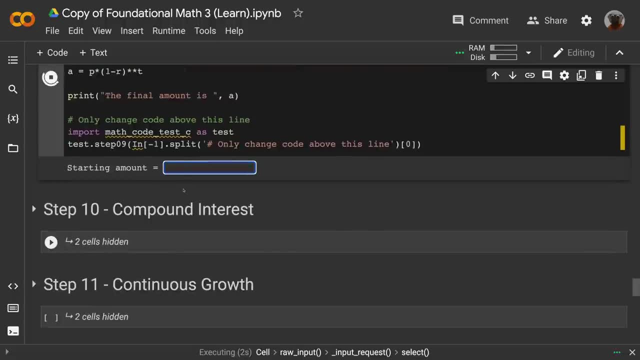 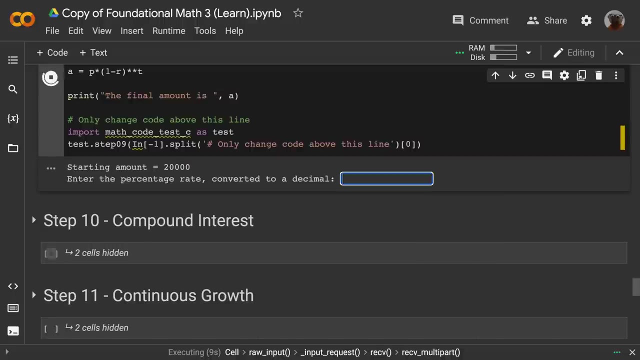 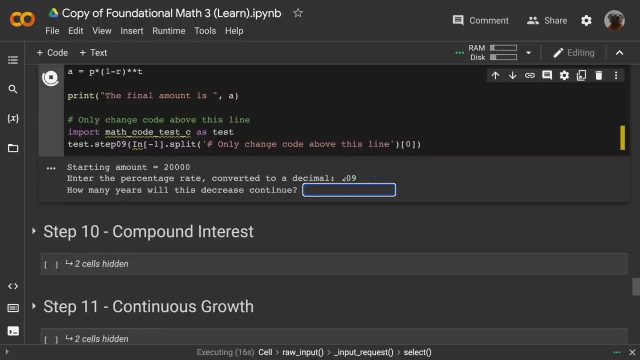 Notebook, The Colab Notebook, Always Wants To Give Us Tool Tips And Advice On What Variable And Everything. So There We Go To The Number. 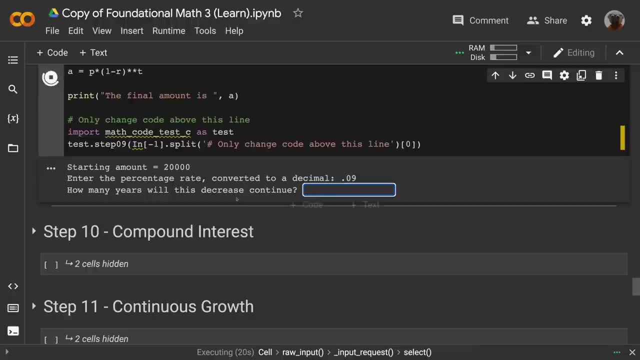 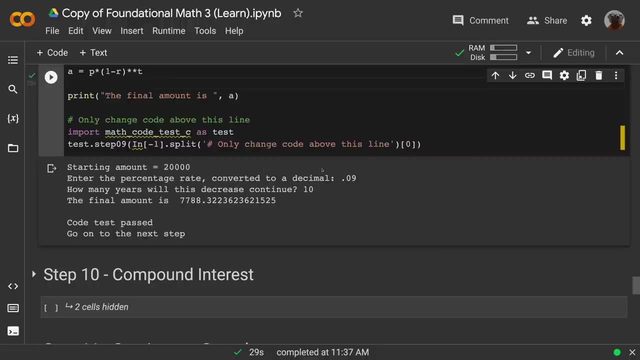 Of Depreciations Which Might Be The- You Know- Rate Of Decrease. Who Knows? And Then, How Many Years Will Decrease? You Know, Let's. 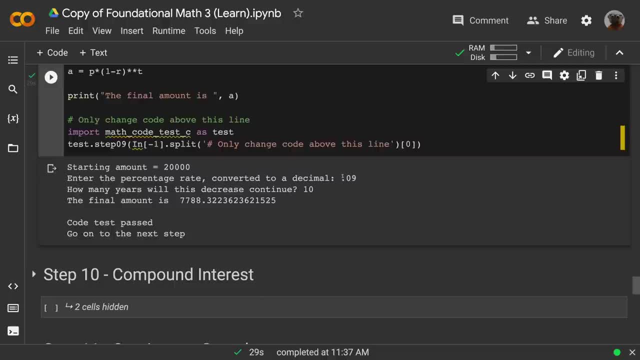 Just Say Ten. So Here For Ten Years. So Then, Ten Years Later, That Car Is Worth Seventy Seven Hundred Dollars, Seventy Seven Eighty. 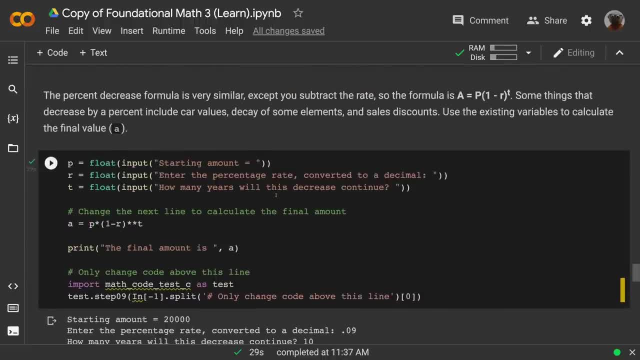 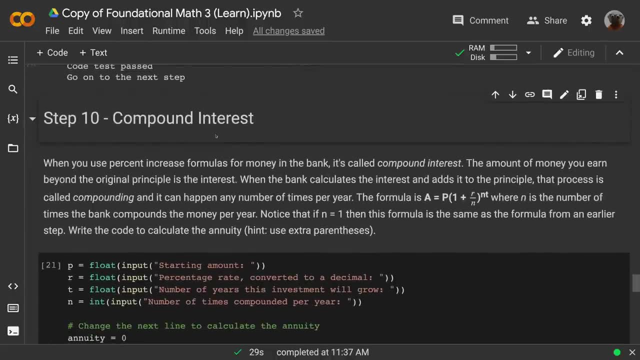 That Might Be The Case. I Mean You Know, You Know That, You Know That Is One Year If It Is Compounded Once A Year. 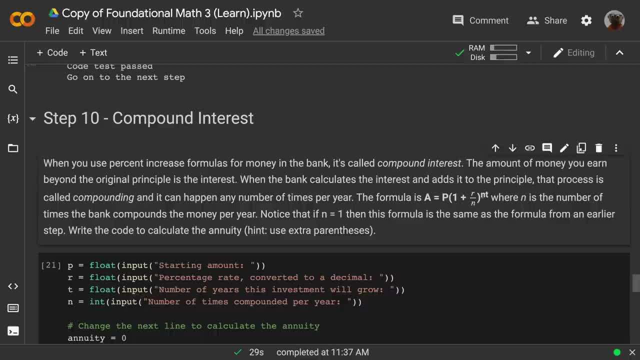 So Now We Have This Formula, Notice How Similar It Is, But It's The Formula That We Would Use And Remember: That's, That's Really. 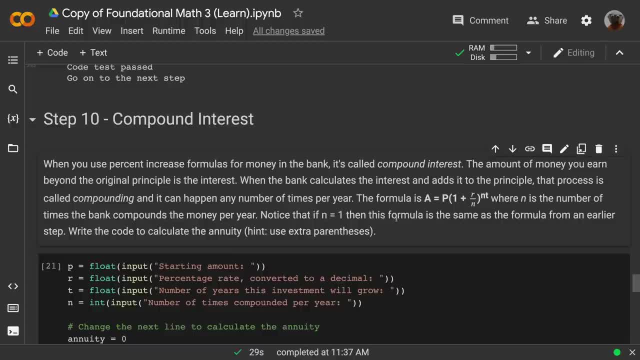 And That's Why We Wanted For Any Percent Increase. That's Why We Wanted To Convert It, To Crucify The Number Of Times We Are. 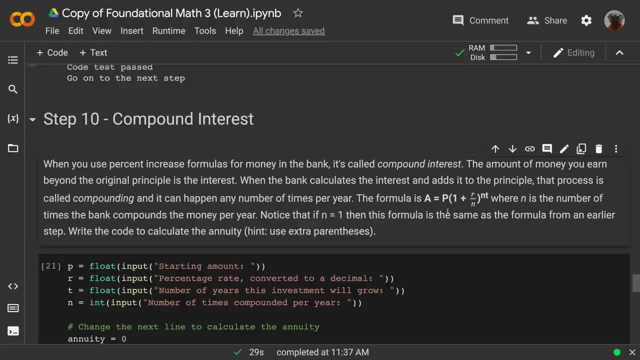 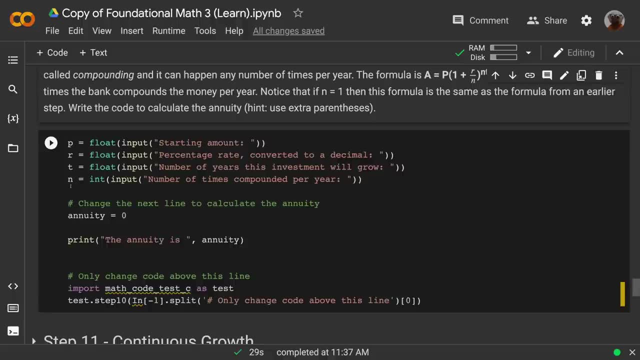 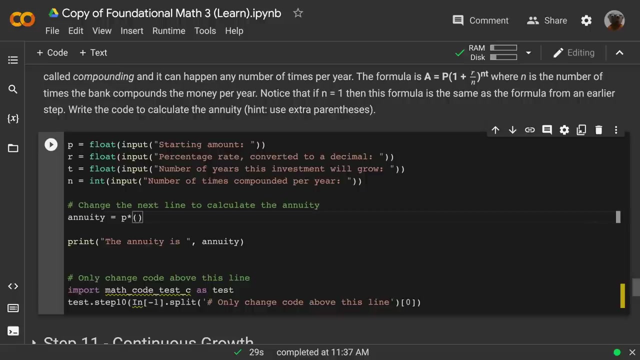 Calculating This Every Year. I Mean N Being 12.. That's Pretty Common. You Know A Lot Of Banks, A Lot Of. We'll do p times and, in parentheses, 1 plus. 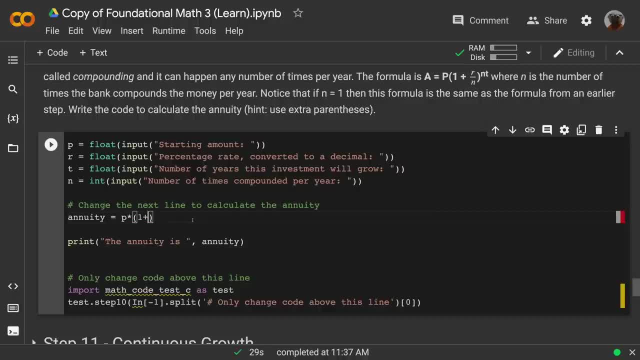 But now I have r over n, I'd rather use extra parentheses just to make sure that nothing gets mixed up in the math. r divided by n, And all that to the. So you see r over n in the extra parentheses to the nt. 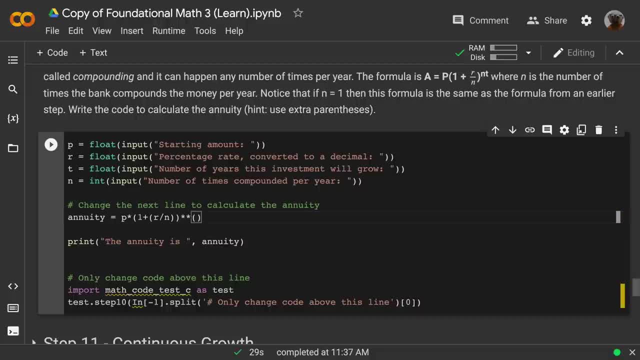 But again, just to be sure, I'll put that in parentheses: n times t in parentheses, So that way it stays together. Python might not, but I want to make sure it doesn't accidentally take it to the n power and then multiply by t. 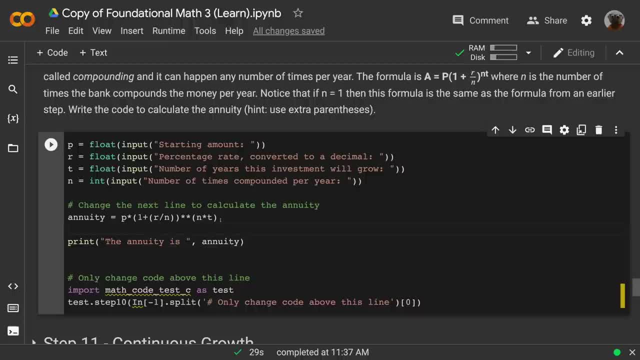 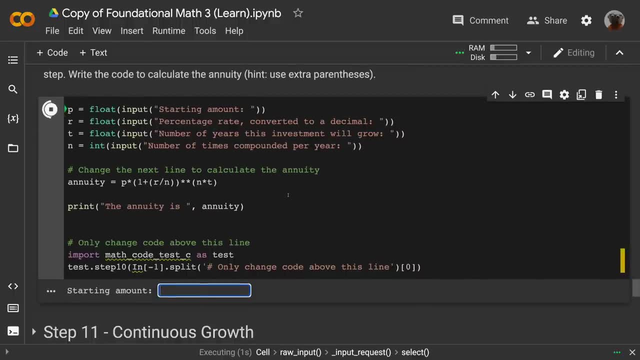 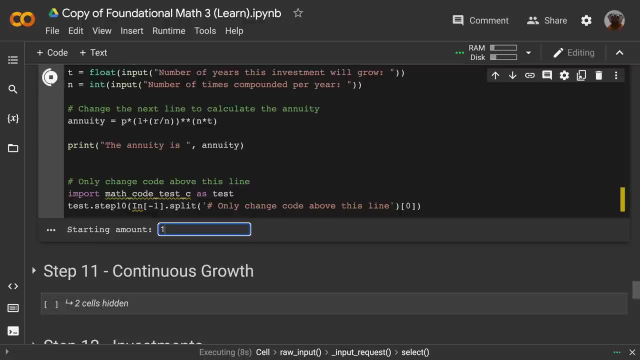 So there we go: p times 1 plus r over n to the nt And that's going to give us our annuity. So just to be interesting, let's use the same one we did two steps ago. That $1,000 converted to a decimal and we were saying that that was at 5%, 0.05.. 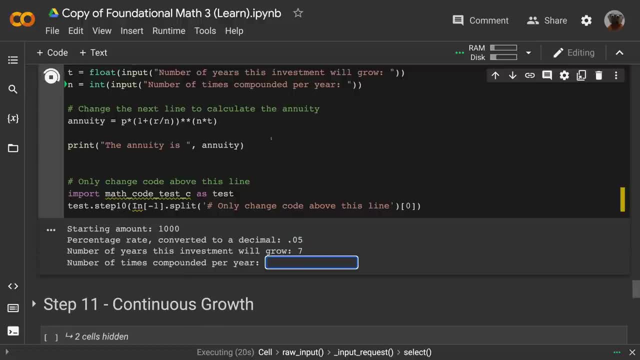 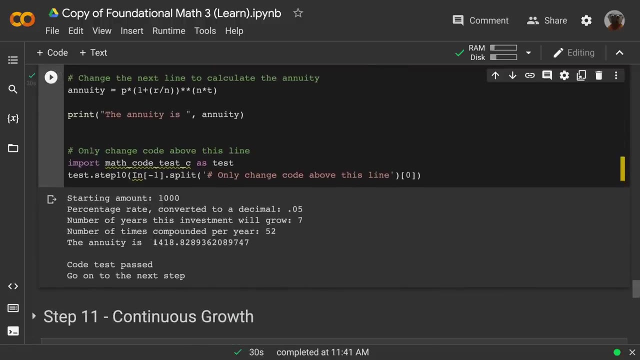 And we said 7 years And 12 is pretty common, but I'm going to say 52. Let's say it was compounded every week all year. So what did we get? $14.18 and $0.82.. 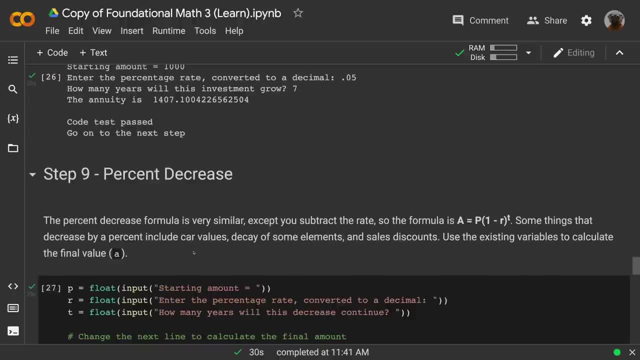 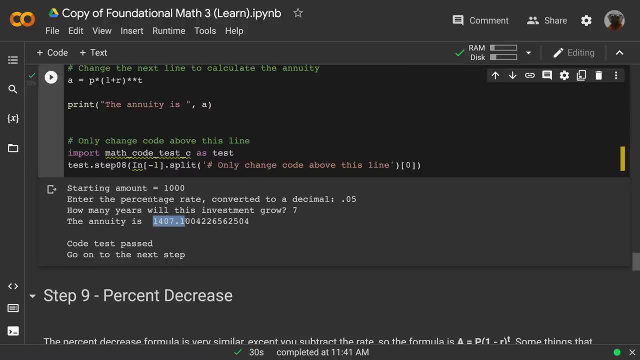 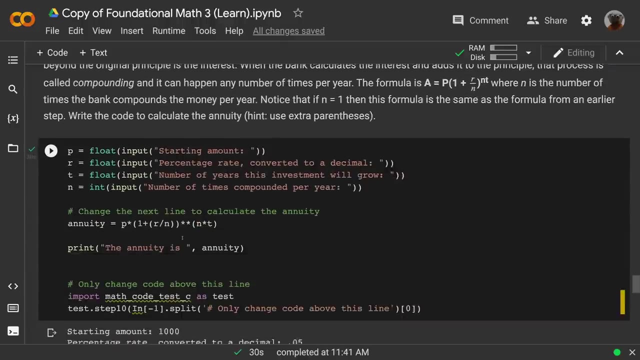 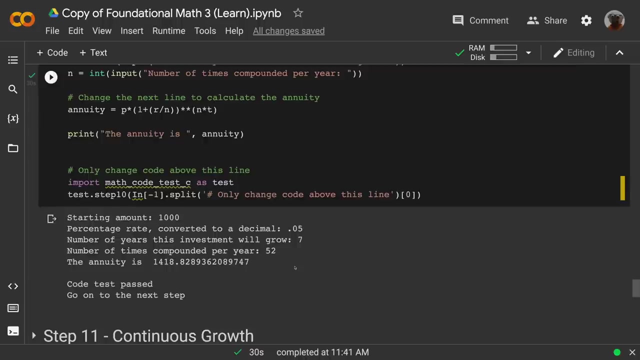 And let's just quick go back and compare this to our increase $14.07 and $0.10.. So look at that, Just that little amount of money made us another $11 because it was compounded. that often It's a little bit more because you have that little bit extra advantage. 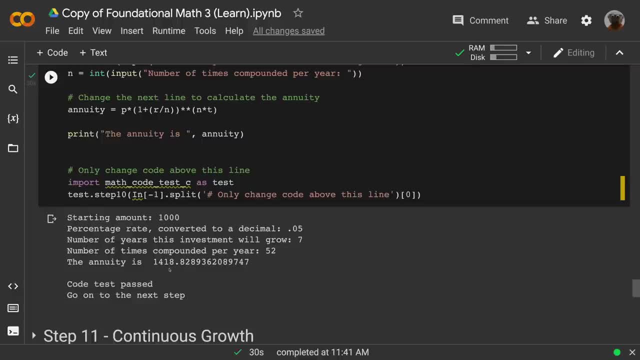 This is money growing. And then that little bit extra percent for that little bit more time gets you a few more dollars. So you might be thinking, well, okay, 52, then maybe 365 would give you a little bit more. 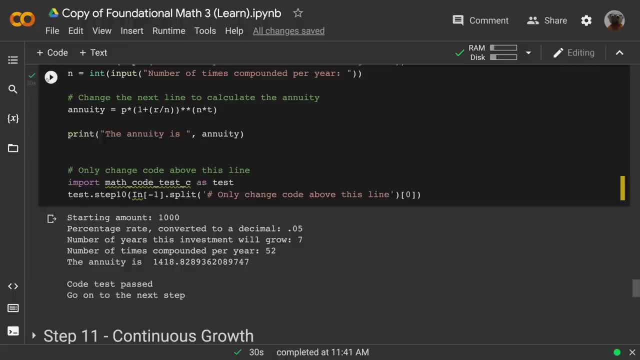 That's true, And we can just quick do that. So remember that was $14.18. And if we did this, so that same $1,000 percent, we're going to do the same: 0.05, the same 7 years. 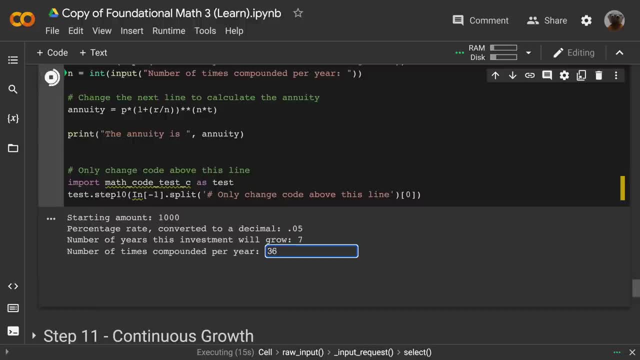 but then this is going to be $3.65 compounded every day, So you see $14.19.. It gives you another dollar. So compared to You know you made about $11 more doing this every week. But from every week to every day, you know, it gave you one more dollar. 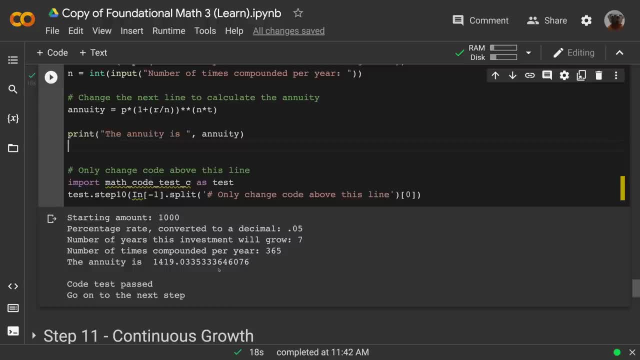 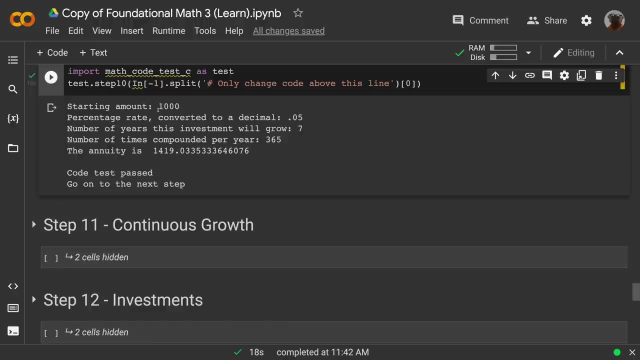 So there is a point to where it doesn't really get you that much more. And then we start thinking about: well, okay, can I compound it multiple times per day, etc. That's when we get into continuous growth And continuous growth if I use that formula. and then 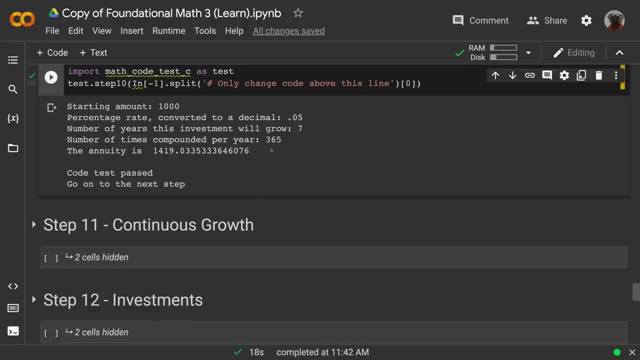 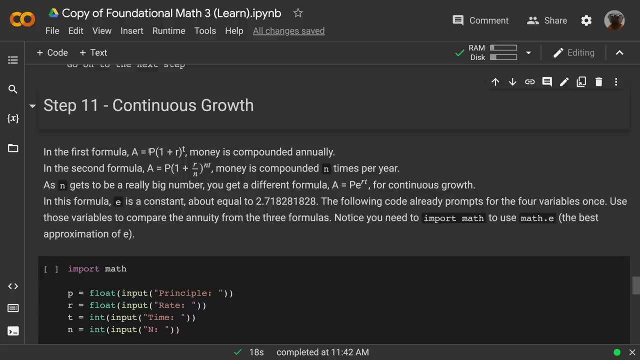 Compounded it multiple times a day, If I compounded that like three times a day and, who knows, maybe I could even make N like an even thousand. It starts approaching this other formula for continuous growth. So to recap, so there you go. 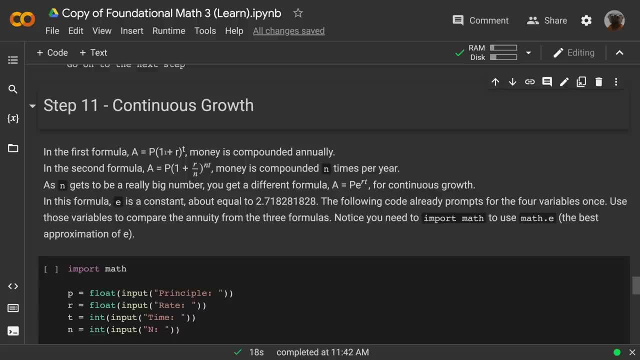 That's, you know, money compounding annually. So that's the percent increase, but we take it as annually, And then N times per year we have this formula And then, as N gets to be really big, like I said, like a thousand or something. 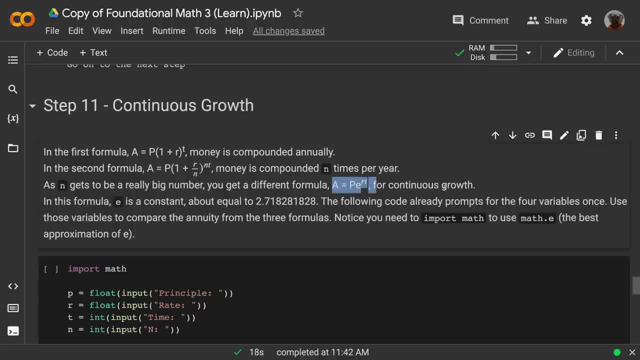 it actually approaches this other formula P-E to the RT And this is useful because, as we see later, better ways to even figure out what the rate or the time would be if I know these other values. So it goes from this a little more complicated to 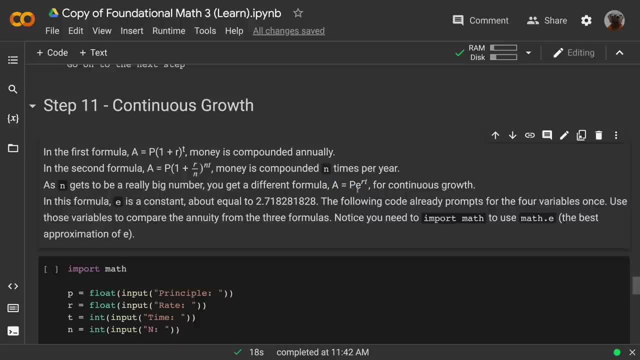 I actually think this is a little bit easier. formula P Times E to the RT And that E is not just a random variable. E is this constant equal to about 2.718281828.. That 1828, after looping through that twice the next time, it's not exact. 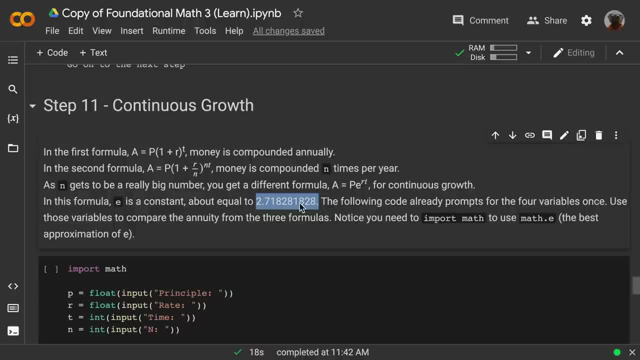 So it's not just like this: you know, keeps repeating. That would make it even easier, but it actually after that second time, then it's a little bit different. Okay, so we give the code that we're already going to prompt for these. 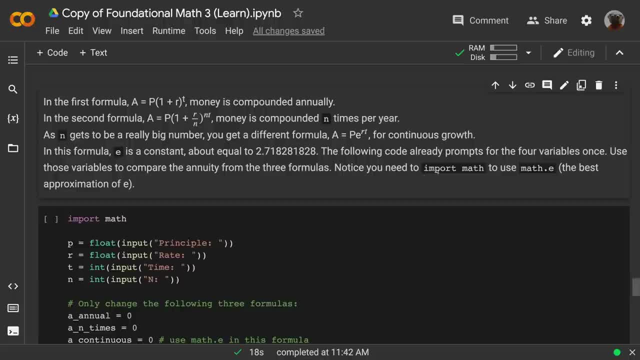 And this time we're going to add one more import statement. We're going to import math so that we can use mathe. You know, you don't have to worry about typing in this, because actually mathe is going to take it to even more decimal places. 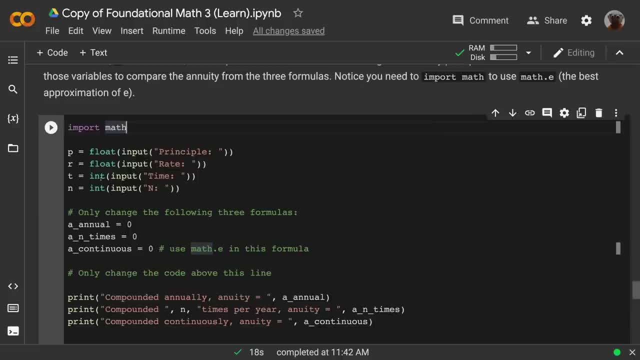 So we have the same thing here: Principal rate time And Um, There you go: Time, And that can be an integer. That doesn't have to be. It can be an integer or a float. Um N is going to be an integer because you can't like. maybe you know. 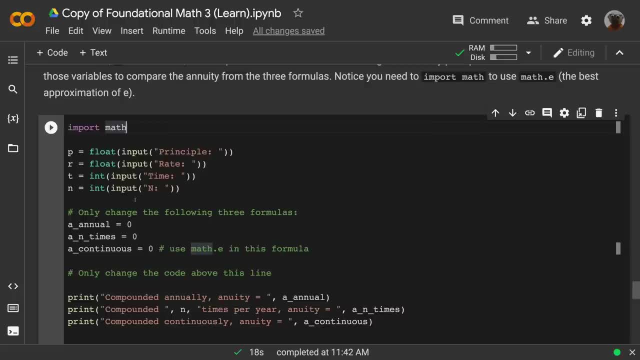 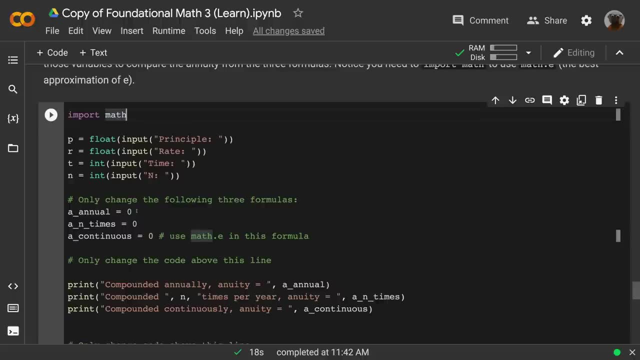 how many times did you compound it? You can't say like, oh, one time I kind of like halfway did it. That doesn't work, Okay. so now we're going to use these same formulas we did before. 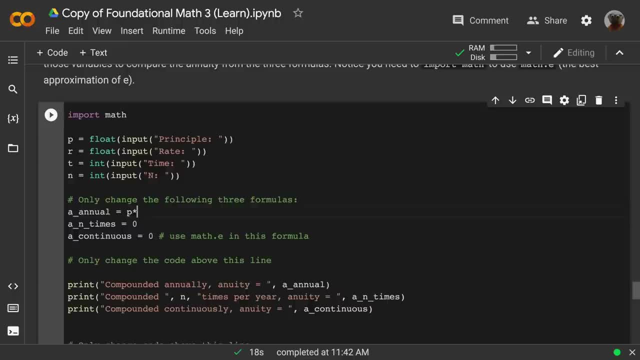 Annual. So that's going to be P times Uh times one plus r, exponent t, Just like that first formula. And then this one is going to be P times one plus the extra parentheses r over n. All that to the exponent of nt. 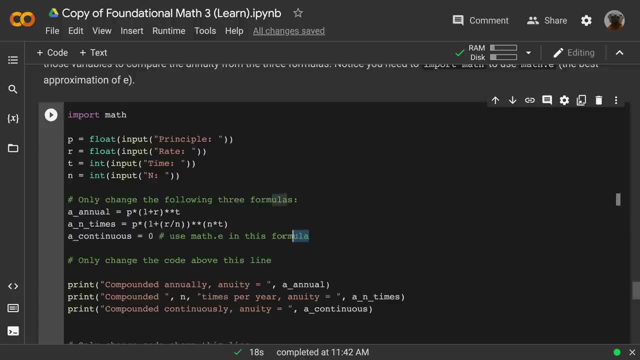 So these are those two formulas, And now this one, we're going to use mathe. So that's going to be P times mathe to the exponent of r times t. So there we go, We see P e to the rt. 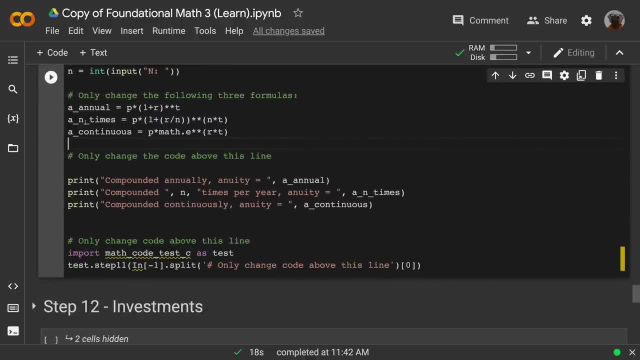 And now we have these three, So we can prompt. And let's, Let's compare these, Compounded annually, Compounded n times per year- I'm going to put an extra space in there- And compounded continuously. So let's take something here. 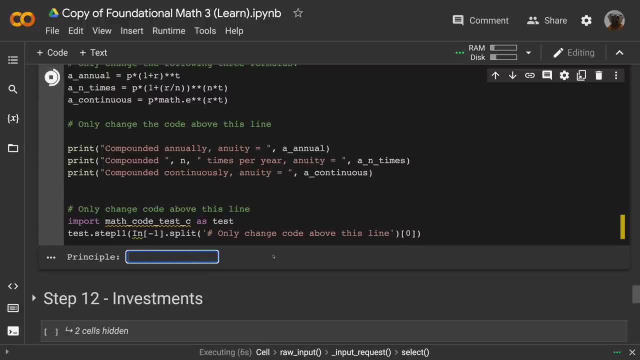 And let's just say a principle of There we go, So 11,000 rate, 0.0.. 6.. And time, And let's just say, you know, 15 years, n, And we only need that for one of those formulas. 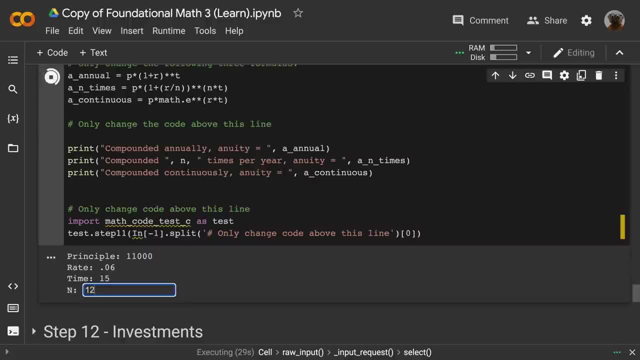 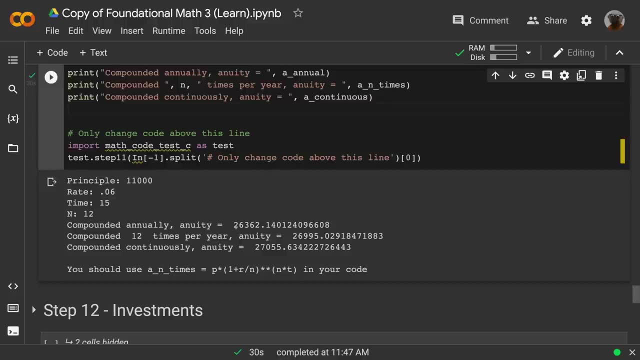 But let's say n is a normal 12.. So, given this, compounded annually, you would have this much: 2632.. Compounded 12 times a year, 26,995.. So, wow, that made you know more than 630 more dollars just by compounding it. 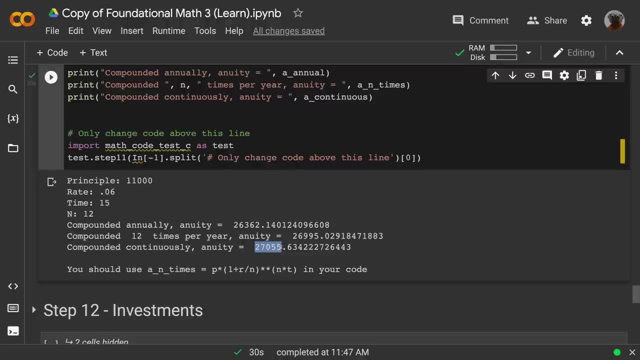 But look at that, Compounded continuously 27,055.. So there we go. Yeah, So you see, from here, from once a year To multiple times, we're talking about making you know more than 600.. 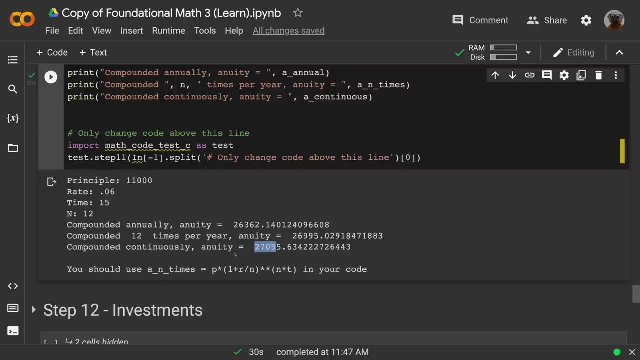 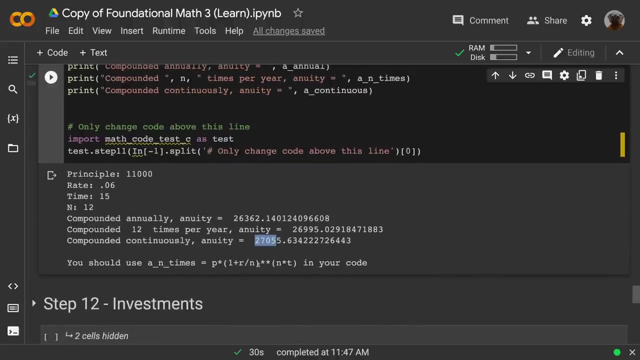 But then from that to compounding it continuously, you know, compared to the original, you know we're up to about $700 more And it kind of evens out that Oh, And this one I think I, I 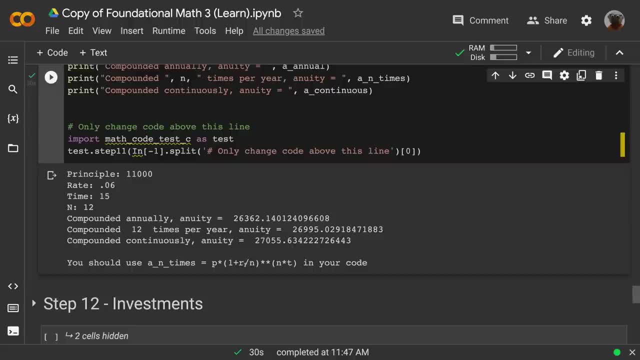 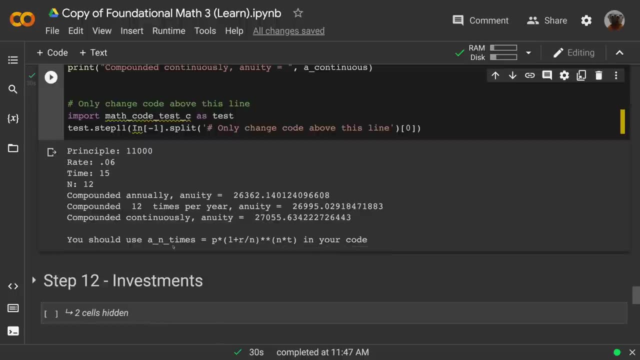 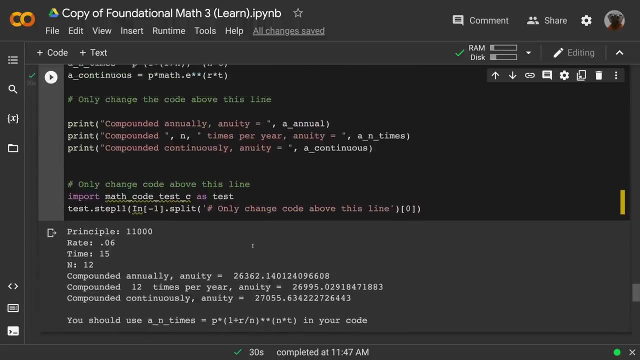 It gave this error because I used the parentheses. So if you're going through this and if you know, you know these errors messages are supposed to be hints, just to help you out. So it was without the parentheses And that is okay, because Python does no order of operations. 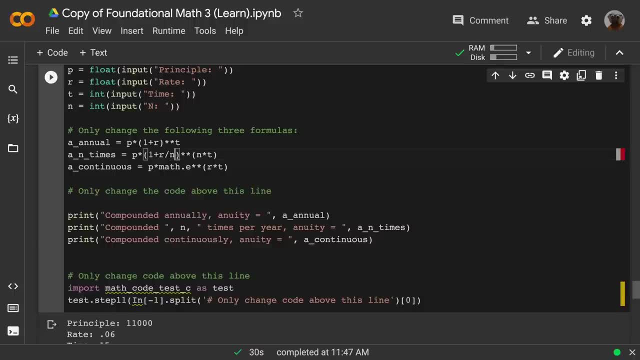 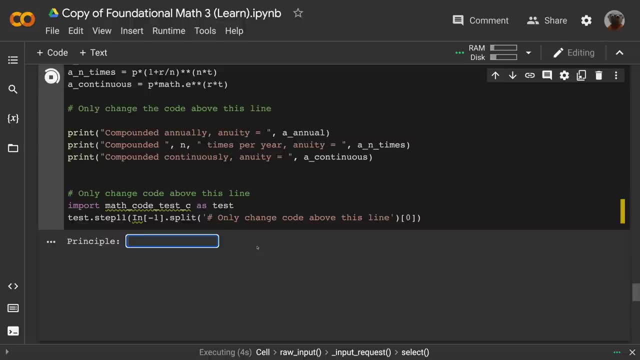 But without the parentheses. it should give us not the error. So There we go And should give us the same values here. So 11,000 rate, 0.06 time 15 years, And we said it was 12.. 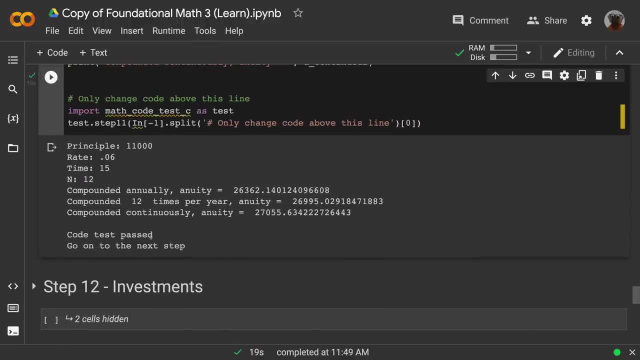 So we see same values and the error message saying: you know- maybe I'll go in and change that- that the parentheses are okay, All right. So there we go, Prompting once and comparing these three different ways of calculating interest. 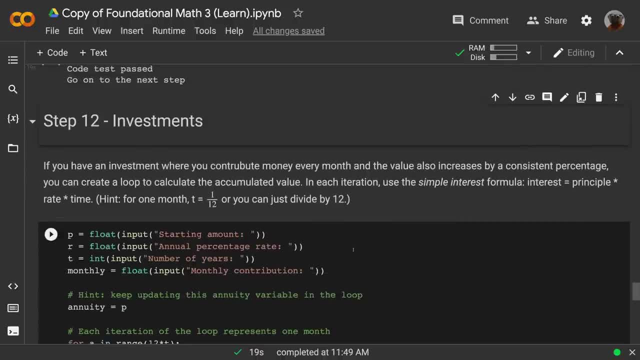 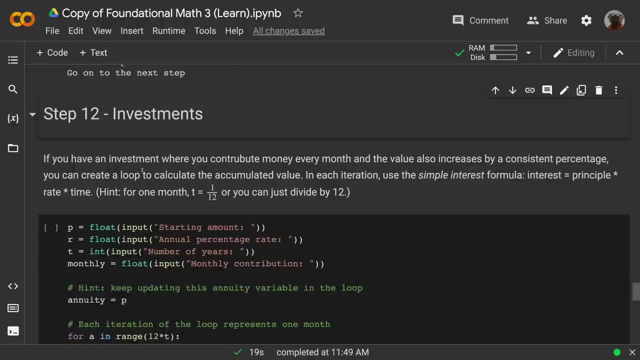 So now some of this comes in where we have, you know, some investment here And investment often. you know something you might be contributing to for retirement And you have. You have some accumulated value. So we have any of these formulas, but we also contribute money every month. 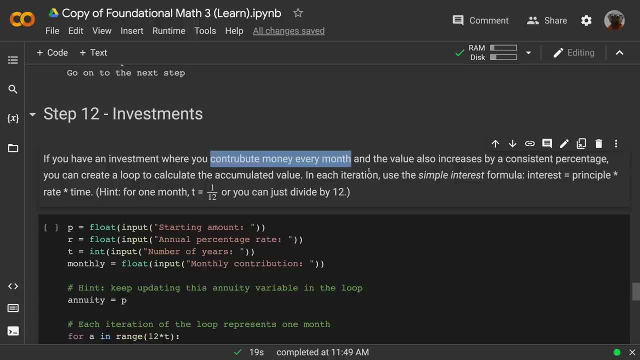 And this I will say month, monthly. That's kind of a normal, normal thing, So I'm not going to worry about, like all the different values that that could be Okay. So we have something that's going to increase by a percentage and we're using just that simple interest formula. 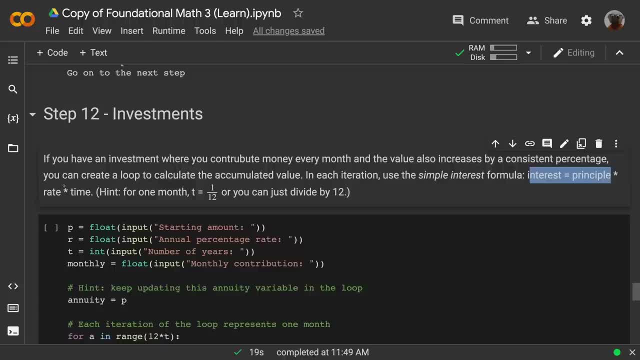 Interest equals principal, times, rate, times, time. So that is just simple interest. but for one month that works out, And for one month t equals 1 over 12. Because time in years, but then over 12. You can just divide by 12.. 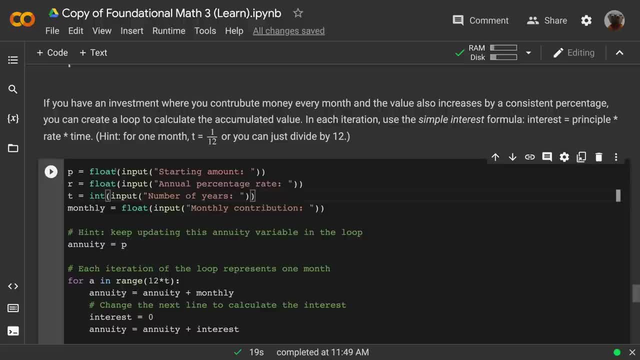 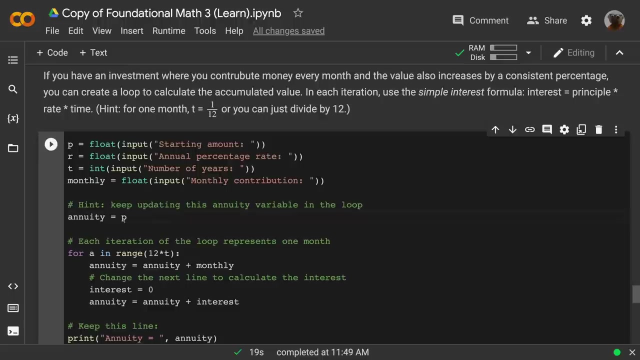 So here, if I have this, we can set up a loop here. So, Um, PRT, but then monthly we're going to ask for the monthly contribution. All right, Now this annuity: at the beginning it is P, what do you have? 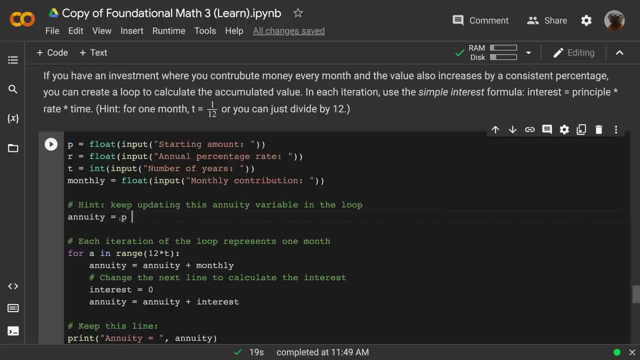 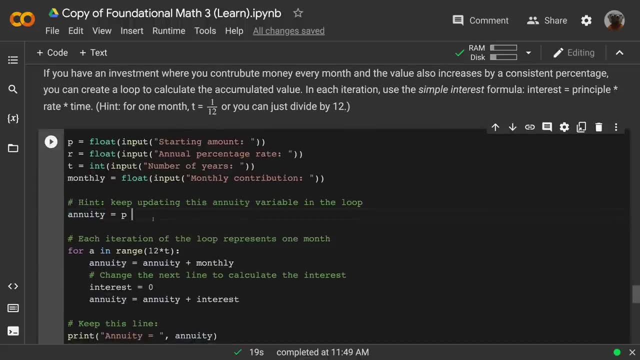 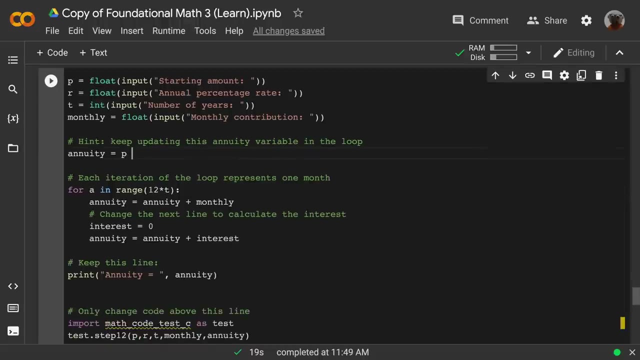 I have this, I have this amount done, So we'll keep that, but it's the it's the annuity variable that we're going to keep updating. So somebody said time in years, So then our loop is going to be 12 times T. 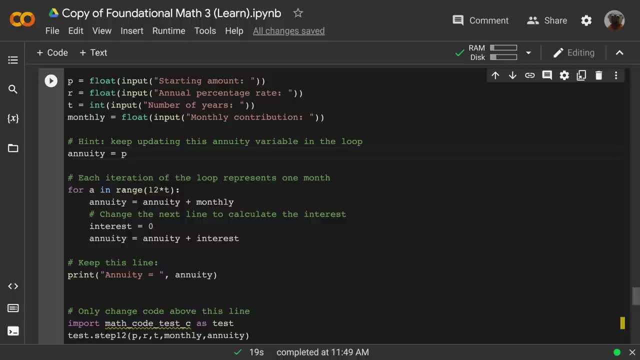 So monthly contributions for this law for A in range 12, T. And now let's see. we're just going to say, first of all, the annuity equals annuity plus monthly. All right, So now that annuity value is greater, 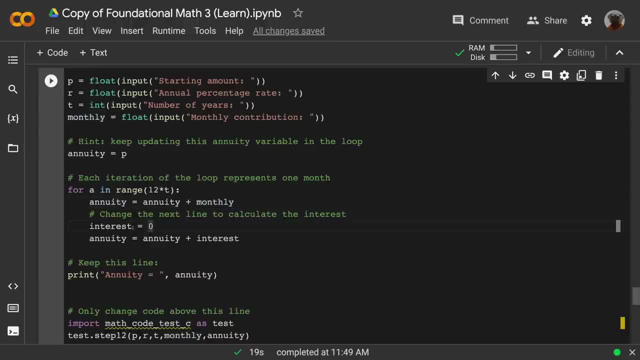 And then now we want the interest, Just the interest. So that's why simple interest is just the interest equals, um, annuity, which is the times rate, time, uh, and then times one over 12.. And I'm just going to say: divide it by 12.. 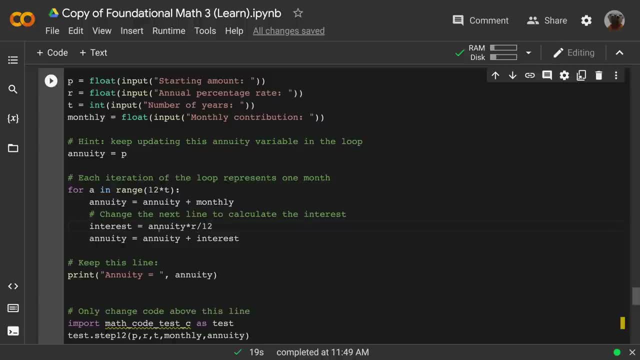 So we see that in principal times, rate, times, time, and then one 12th is divided by 12.. So now we have just the interest, And now again I'm going to update annuity. annuity equals annuity plus interest. 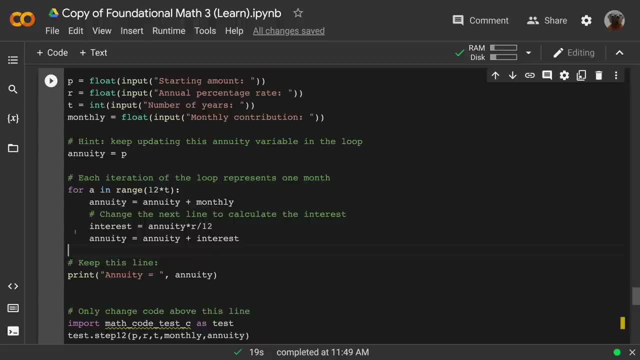 And because I'm making this a loop, then, uh, you know these other formulas are useful for not having to do a loop, but we also wanted to add in this contribution, And then there we go. So you know, we have a few things going on in this loop. 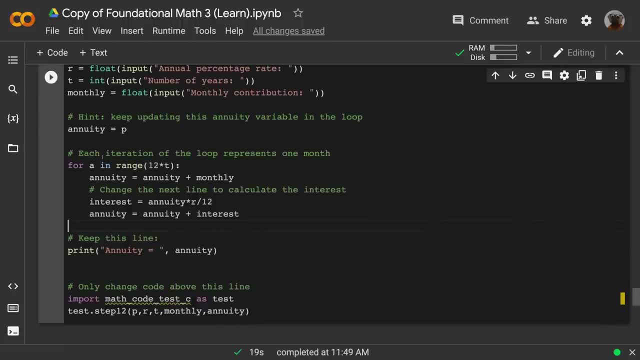 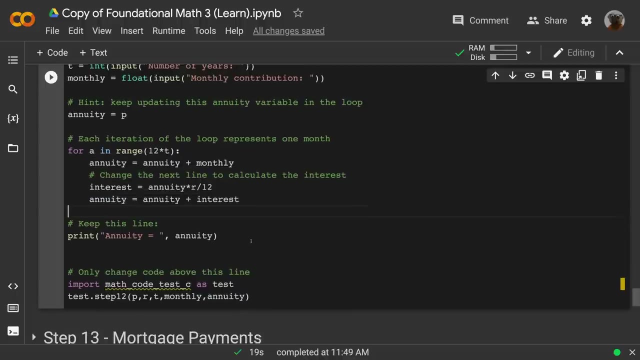 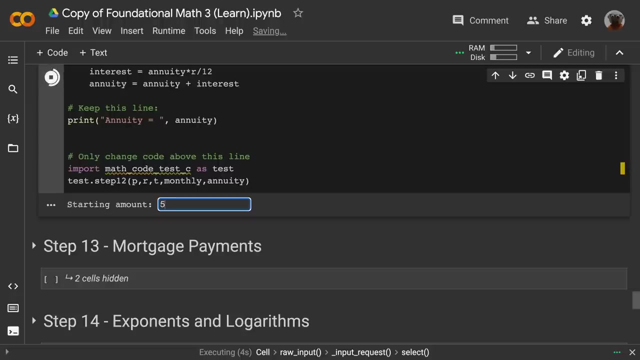 And then, after all the loop it's going to go through and each time you know, add the contribution, Increase it by that percentage for that little bit of time you know now, update annuity and keep going. So when we have this so starting amount, maybe we can say 5,000 and annual percentage. 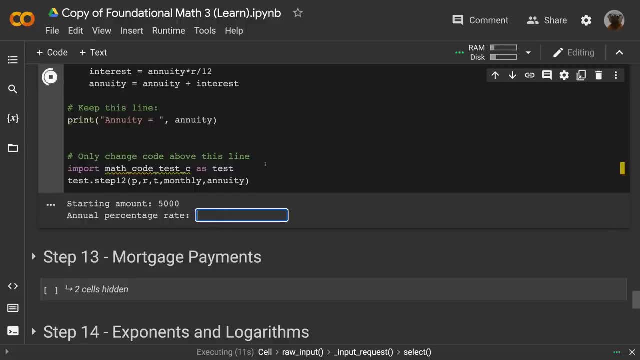 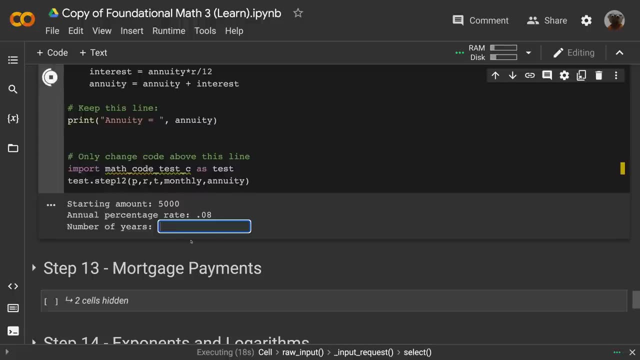 rate. Let's be optimistic, for you know some, uh, you know retirement account: 0.08.. And then number of years. but then these are some of the things you might contribute and then have it, uh, grow for years. 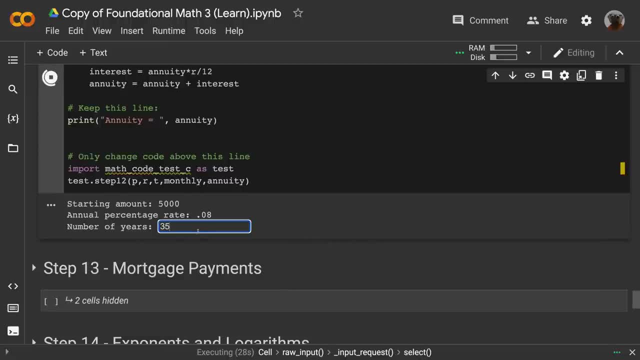 So we can even say something like long amount of time- 35 years- There we go. Monthly contribution, So let's say like 400.. There we go. So that's, that's what we have. We start out and then every month you're contributing 400. 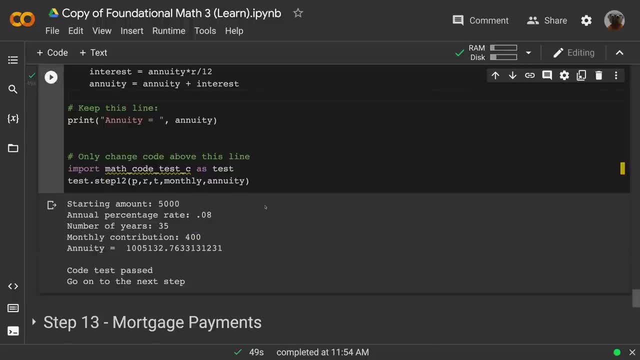 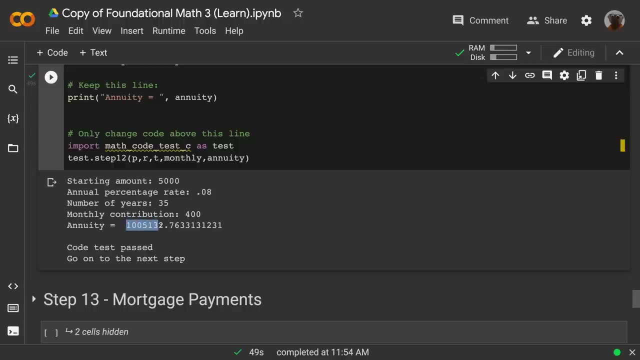 And it you know, we hope it's growing at that rate. So, given this notice, how notice what this number is? that's a million dollars. So what this is saying is etiquette. some of these the the rate it it changes. 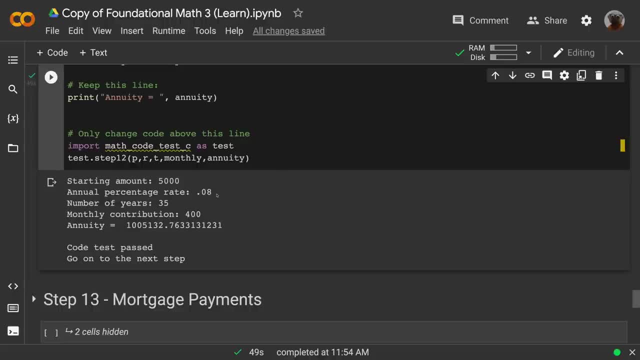 That's, that's a good estimate, but, um, it's a reason to very reasonable estimate. So, putting money away, you know, start working, Put $5,000 away and some good account, or as 8% for 35 years. 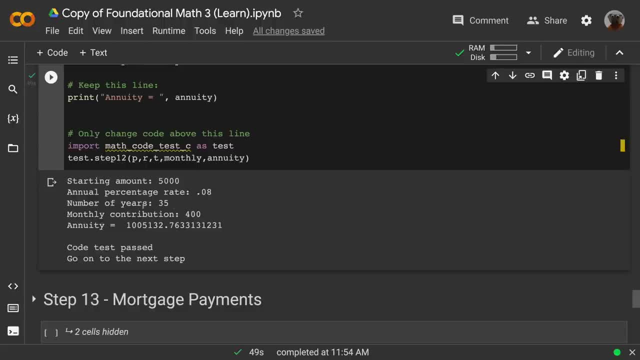 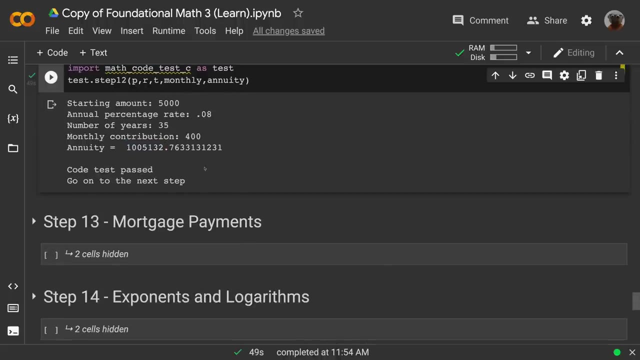 And then each, you know each, each paycheck you're contributing, contributing money. Then you retire with a million dollars. There you go, Things to think about that you can put away this little bit. forget about it for 35 years. 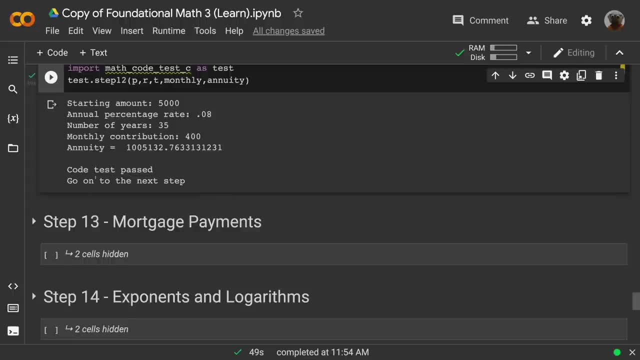 We'll not forget. But you know, and you know, have this, because if it's earning, if it's still is earning- 8% as a good estimate, 8% of that million is $80,000.. And that way you know $80,000 interest. you can live on that and it still has the million dollars there to keep generating more interest. 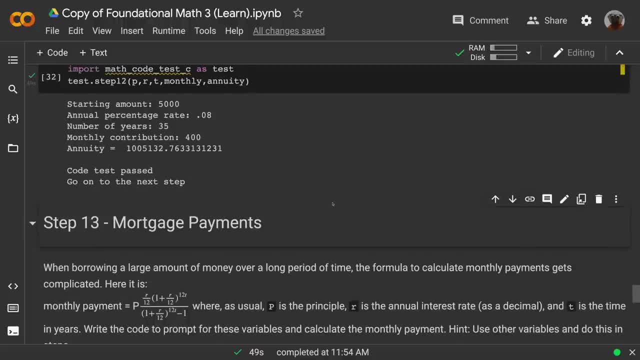 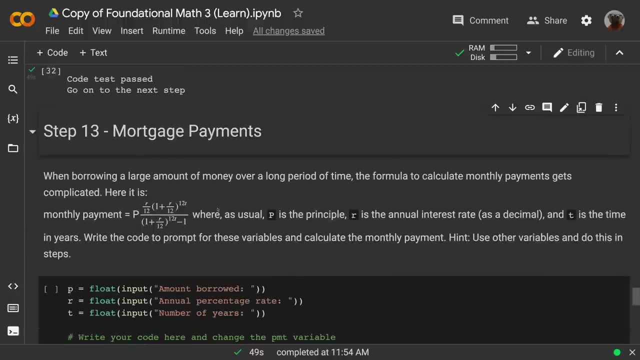 So there you go. Okay, So we go from the positive saving money and having having a million when you retire to mortgage payments and, yes, more. um, like the word for death. um, somebody originally coined that as the. you know, like this death payment. 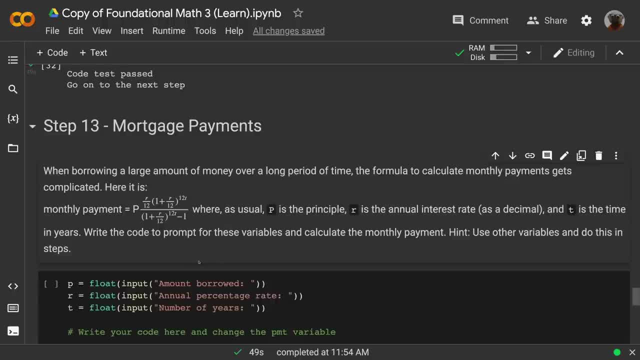 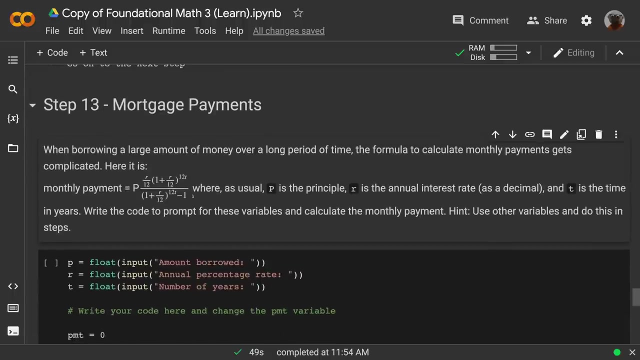 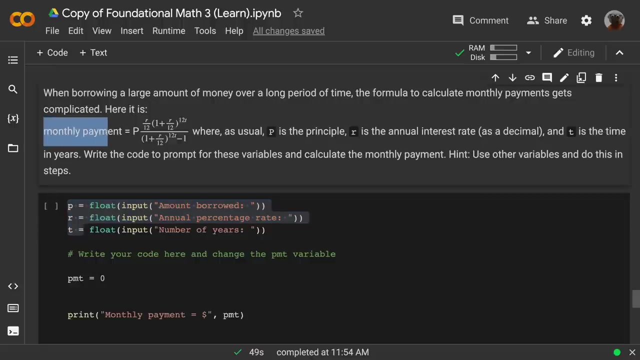 Um, but nonetheless, mortgage for any large amount of money over a long period of time, those other percent increase formulas won't quite do it, Otherwise you, you, you will end up paying a lot more than is reasonable. So this is the much more complicated formula, but remember, that's the value of you know setting these up and writing the code that you, you don't have to like. remember this formula, or you know, plug the numbers in every time you can again prompt for, just like we were doing before, PR and T, and figure out what your monthly payment would be. 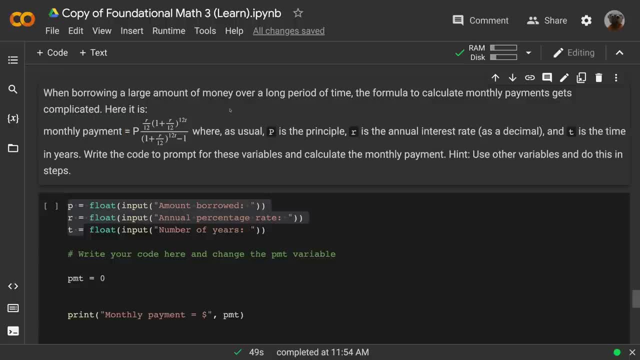 So, given that some large, some huge amount of money and how Banks will set up your mortgage, That's um something else. but knowing how much you're going to borrow and then being able to just run it through this formula and figuring out what would your monthly payment be, that's going to be very useful. 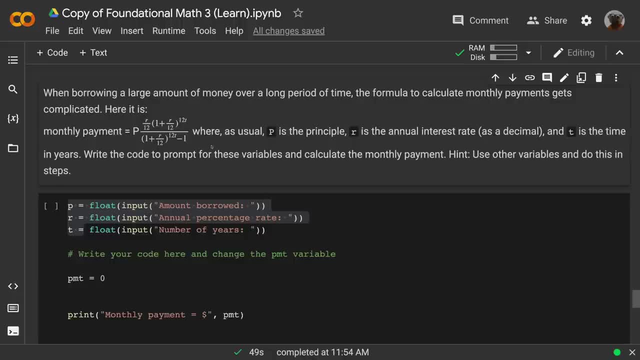 You and again this applies to mortgage or possibly car payments, because that's also large enough sum and a long enough time that this is a much better formula. You and again this applies to mortgage or possibly car payments, because that's also large enough sum and a long enough time that this is a much better formula. 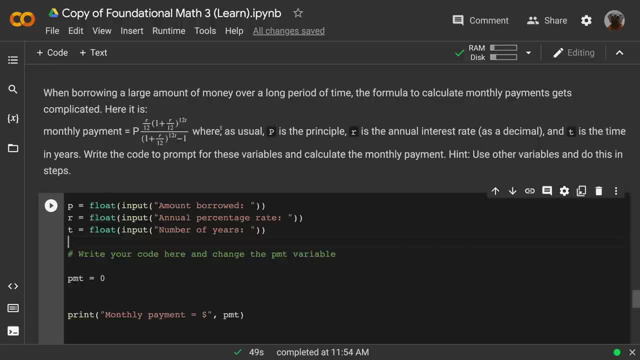 So this is the formula, And again, P is principal, R is rate, T is time, and this would have N there, but N would be 12 each time. And again, P is principal, R is rate, T is time, and this would have N there, but N would be 12 each time. 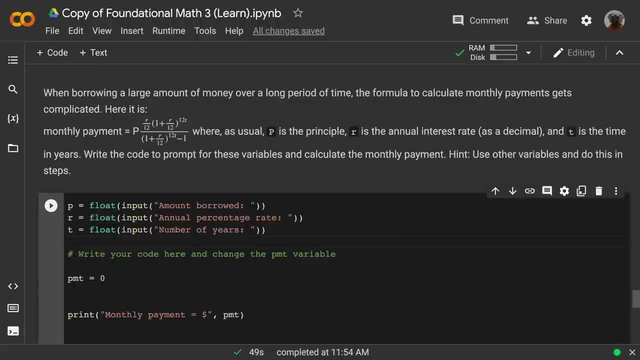 So I just put 12 in there, So it kind of goes along with that formula. but N is 12 each time. You know. there's no other setup. you know daily or weekly mortgage payments, or yearly, No, it's, it's always monthly. 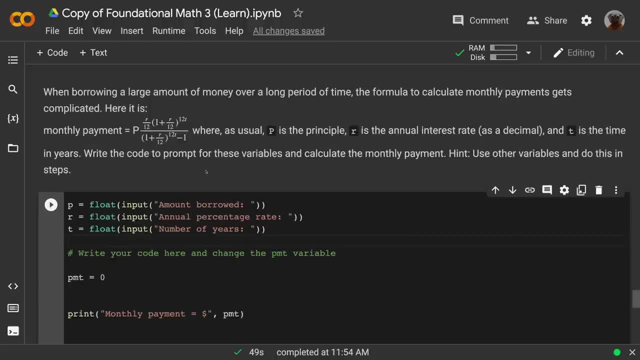 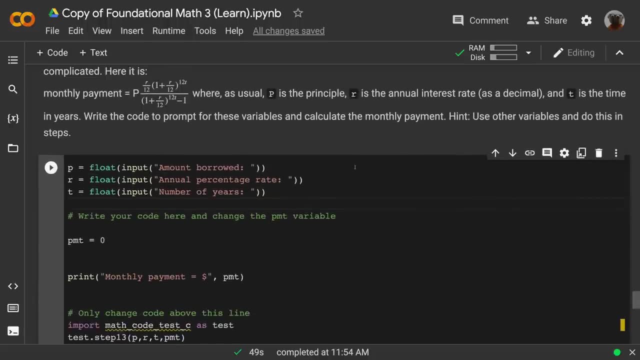 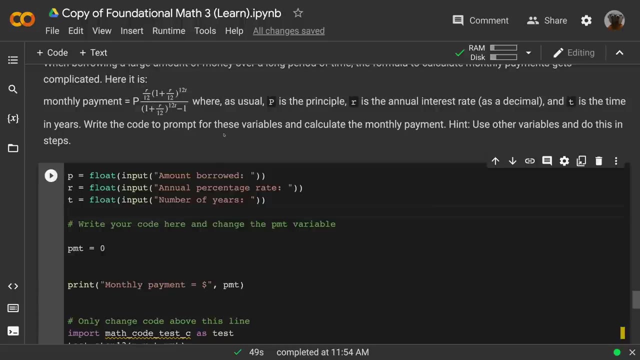 All right, there we go. So we have all these. So Now I gave you a hint to do this- use other variables. I like other variables because look at this R over 12 comes up a few times. So 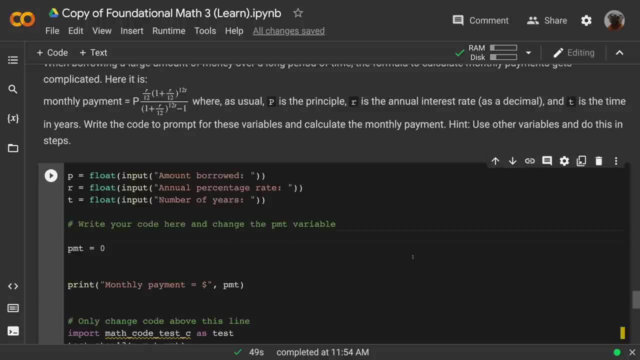 You know we can make this. There you go. R over 12 is a multiplier. Or if you don't want to use other variables, You can do this, There we go. And since I don't have N, because N is 12.. 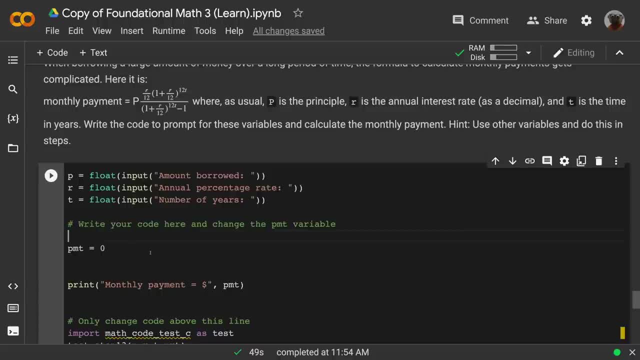 I could have. I might have, like, just like math, N for numerator and D for denominator, And so the payment would be N divided by D, because that just might simplify this a little bit, And then it would be N divided by D. 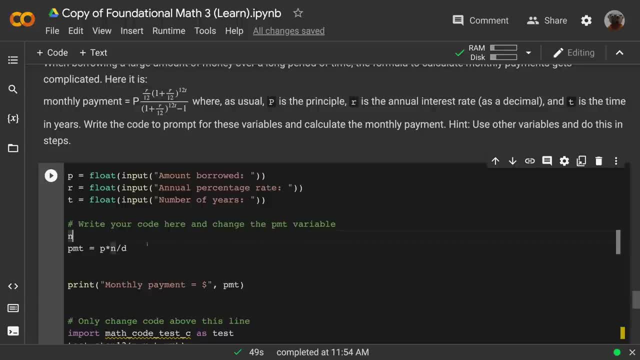 And then it would be P times N divided by D, So I could have just my numerator. So equals R over 12 times, And then in parentheses one over R over 12.. Oh, oh one, Oh sorry, One plus R over 12.. 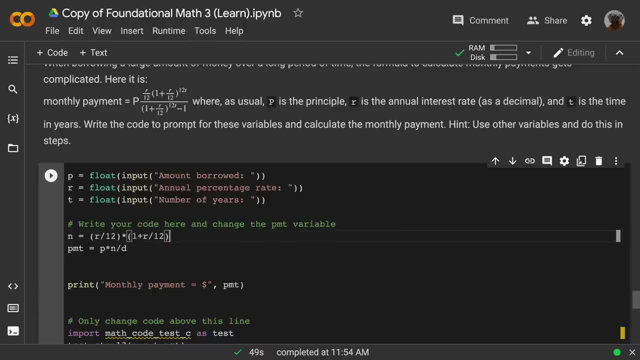 And all that to the exponent in parentheses 12 times T, So R over 12 times one, plus R over 12 to the exponent 12 T. There we go. So that's the numerator, Not bad, And then I can have the denominator. 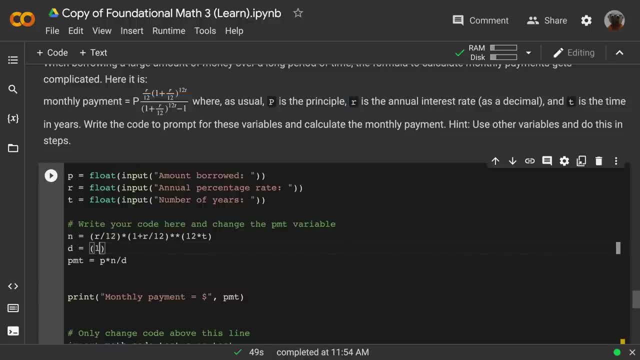 Equals. So one plus R over 12.. There we go To the exponent 12.. I'll put this in parentheses: 12 T, And now when I subtract one, You see, then that's definitely not a part of that. 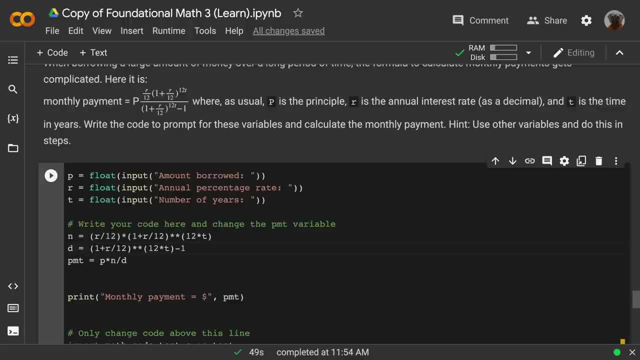 So yeah, And again, you could Add other variables. You can make R over 12 its own variable, or something like that. You could make one plus R over 12. Its own variable. You know different ways to do that. 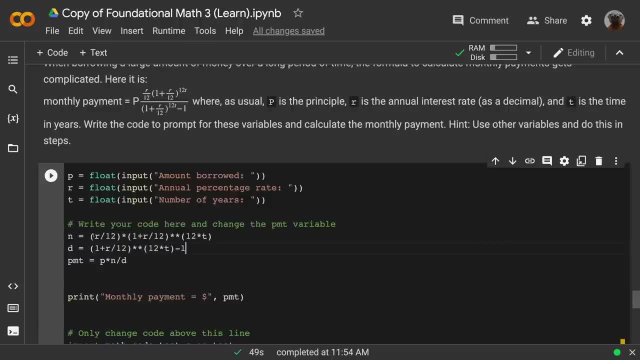 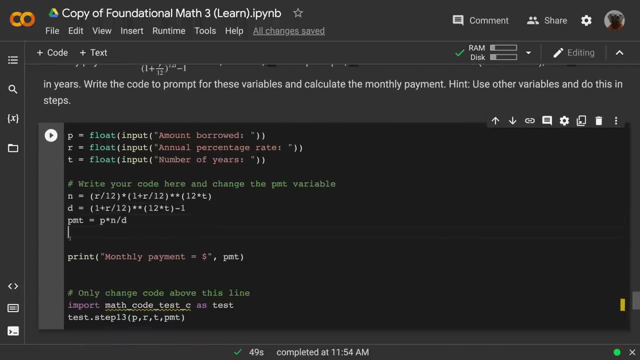 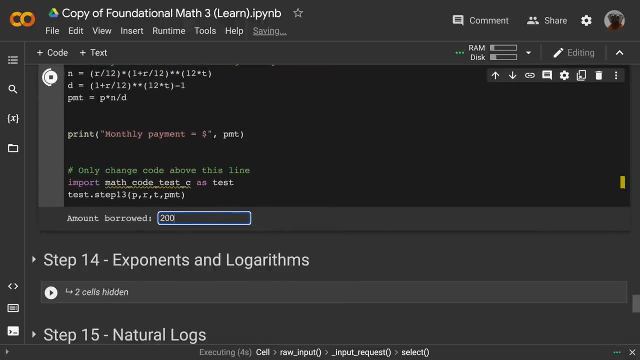 I feel, I felt like this wasn't that bad. So but breaking up numerator, denominator And then payment times, numerator over denominator. So We take a look at this And the amount borrowed we could just say like 200,000. 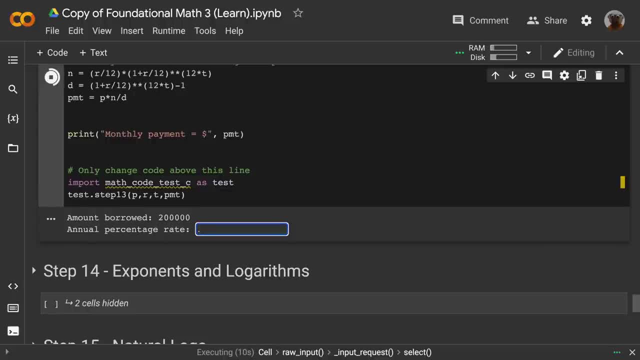 And then we take a look at the For the time being Year Paragraph And then we're gonna go ahead and take a look at the annual percentage Rate. So let's show here the annual percentage rate In here. So if can see the 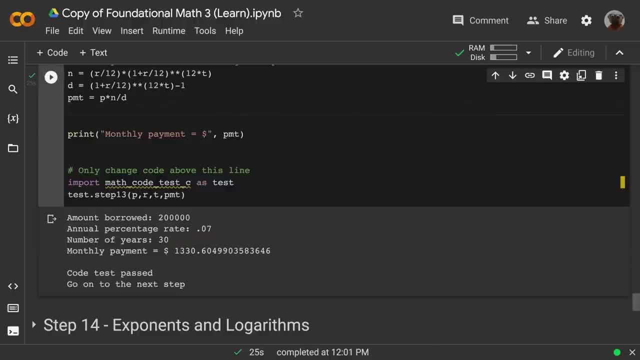 In the data here. There we go. So if, If you're Having an annual percentage rate, Point zero Seven, Yeah, Some of the rates Have been going up, So I'm just gonna say that For now. And number of years. 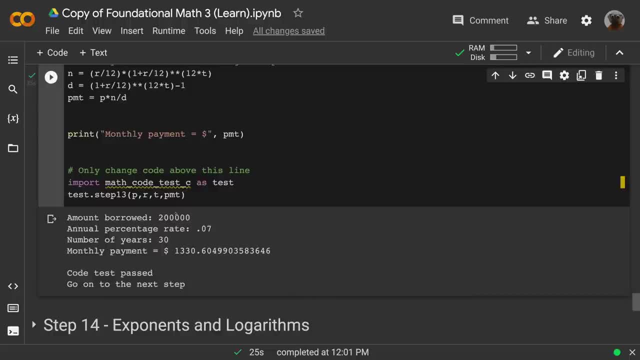 30 is Pretty common, And so there we go. So, So, 13.30. And change. And this helps, Because then you say, Okay, Well, what's the cost of the house? And I have a down payment. You know, you get down to how much you're. 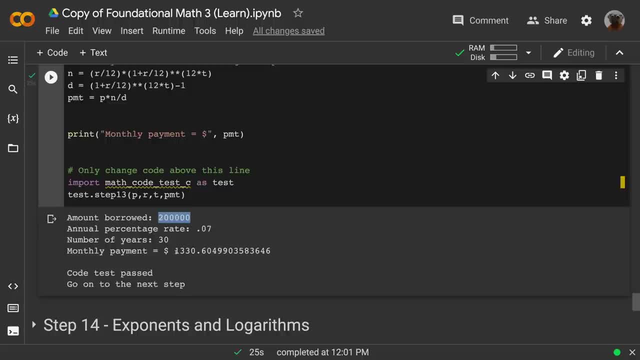 borrowing. That's one thing, Okay, But what's really going to make the difference is knowing this. what would your monthly payment be? That's the important thing, And you know- bonus knowledge- that, no matter whatever your income is, the monthly payment should be for mortgage or rent. 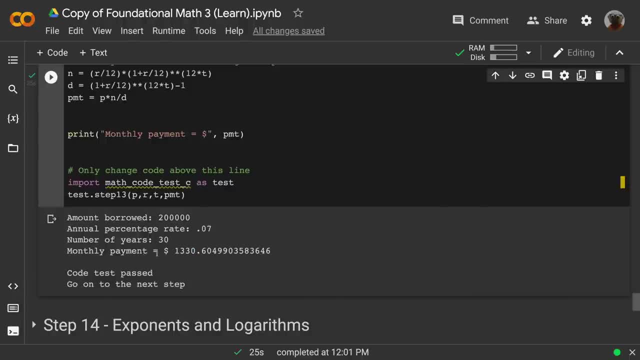 right, It should be one fourth of your income or less. So just to remember, you know, if that's your monthly payment, then each month you should be making at least four times that, Or if you're not, then that's not the right house, Because sometimes you might say, oh yeah. 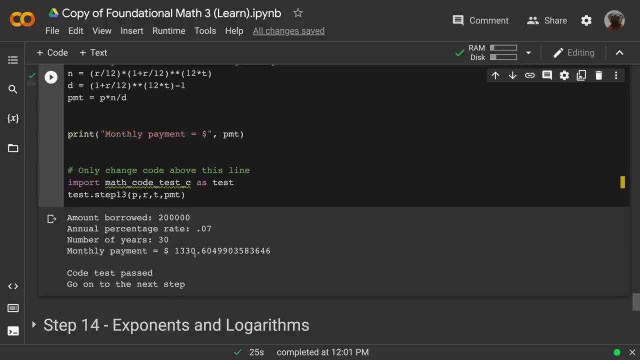 I'm making more than that. I can afford it, But then you end up being house poor. Yes, you can afford your mortgage payment, but you can't afford much else. All right, So let's go. Let's go on to exponents and logarithms. With exponents and logarithms. 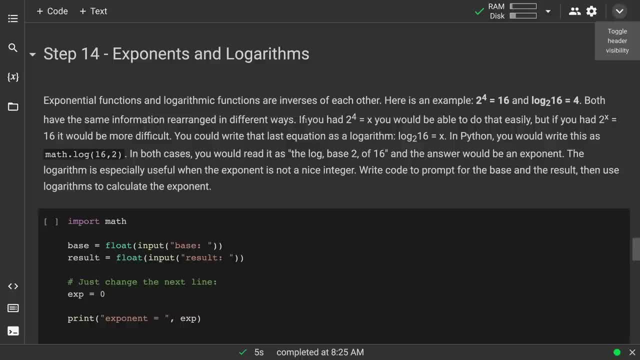 they're inverse functions. They're the same information rearranged. So I have this example here: Two to the fourth power equals 16.. So there you go. Two base two, the fourth power equals 16.. And then the log base: two of 16 equals four. There we go. 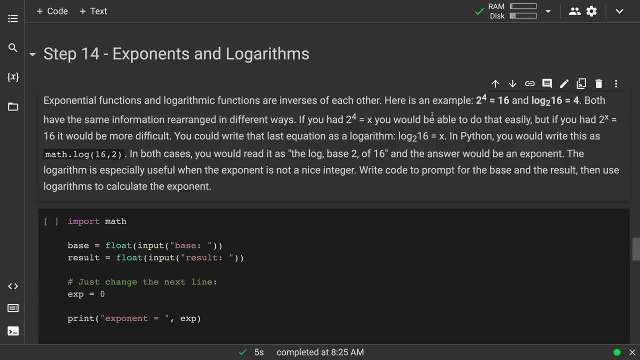 Two of those have the same information rearranged And that's what logarithms are, You know. picture everything on the one side of the equal sign, Oh two to the fourth power. I know how to do that. Plug that into the calculator. But supposing it's the exponent 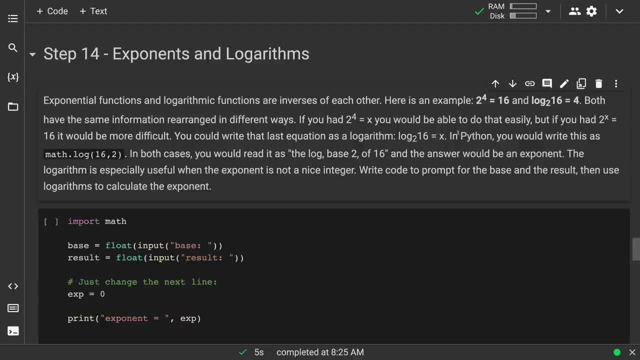 you don't know The log base two of 16.. The answer is an exponent. You know what exponent gets me to that? So this guy, John Napier, like 400 years ago, he realized that that was a missing piece, that that was a situation. a lot of people 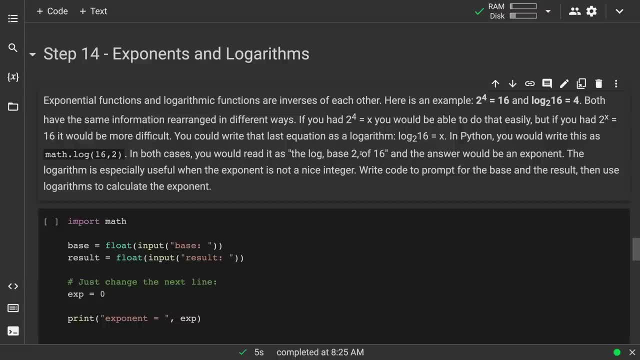 wanted to know the exponent for different things And he spent like 20 years of his life developing this And it was, you know, very useful. You know the original logarithms, it was just books. He could like look them up. Now we have this at the benefit of you know. 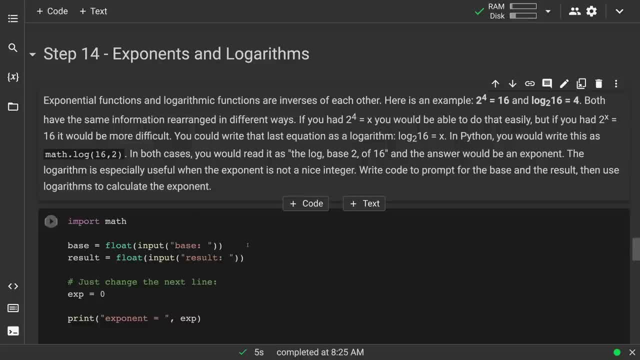 calculator pretty easy And we're going to take it one more. We're going to even write the code that you can just put in a couple of numbers and it'll, you know, calculate it. So if you use the math library- and we'll also look at the numpy library- 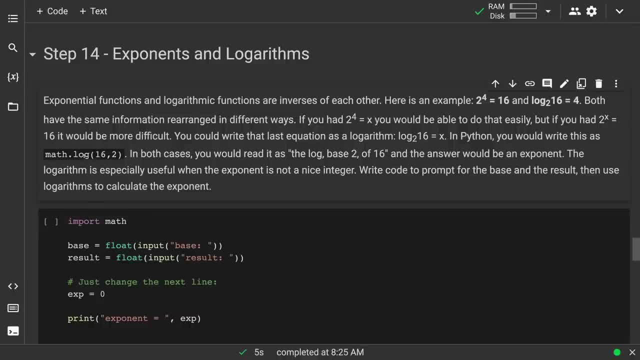 that's another way, But if you use the math library, so it's mathlog, And then the arguments are: you know the log of what, So 16, and then comma, and then what's the base. So there we go. And if you don't have that first argument, 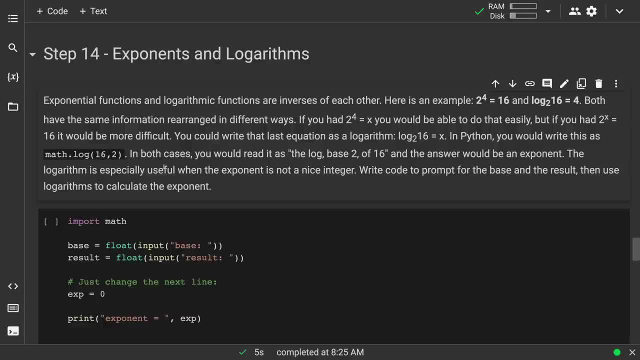 or if you don't have the second argument, if you just say the log of 16, it takes it as base e, But we'll get to that later, All right, so there we go, the log base two of 16.. 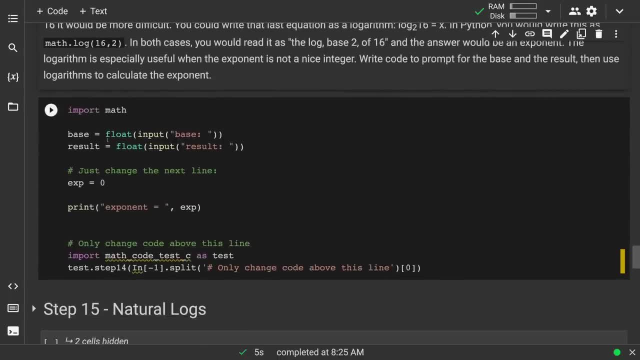 So here's the code. we're going to import math And you know, base, I always call the exponent the result, Just because it reminds me I'm doing a logger and that's what I want. So there we go. So you know, that's the result of. 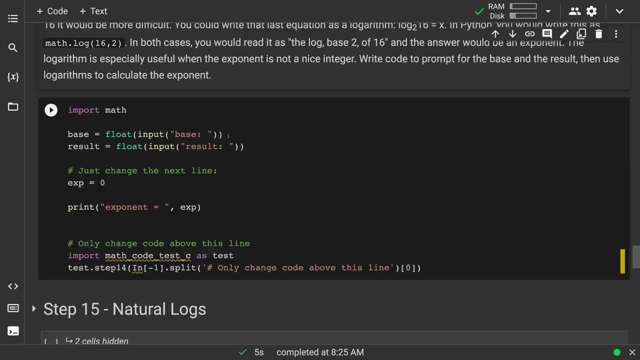 exponential. So as somebody input the base and we're going to input, cast as a float, And the base can be a float, but usually it's an integer And the result and cast that as a float. So what do we want to do? 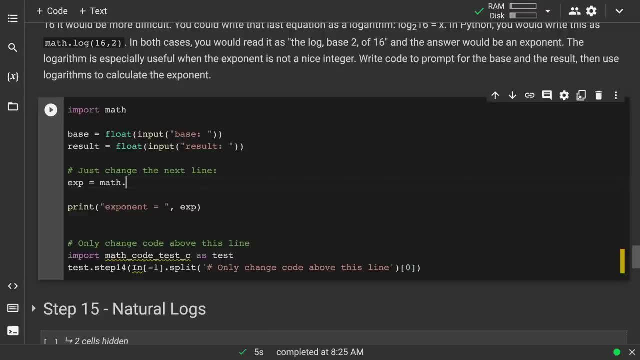 change the next line. Okay, mathlog, And we were just saying result comma base. There we go And it'll import this for it And it'll do this for you. So that's all you needed to do for this And we'll run it And this should check it for you. There we go, Base 27.. 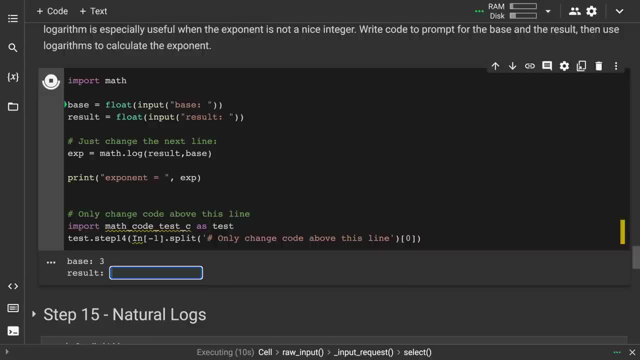 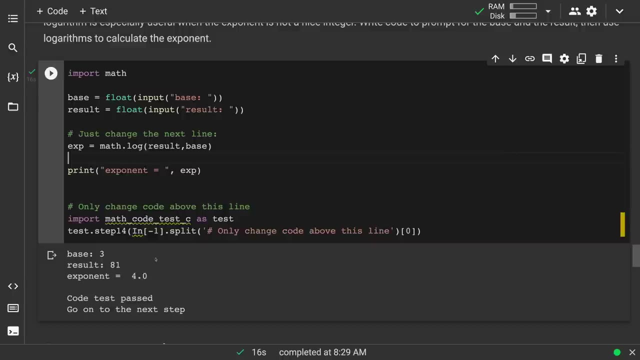 How about this? base Three, Result 81. So it should return four. There we go. So, base, you might be able to do some of these in your head. But if you have, you know base, you know three, to what exponent gets you 81?? All right, you can do that in your head. That's four. 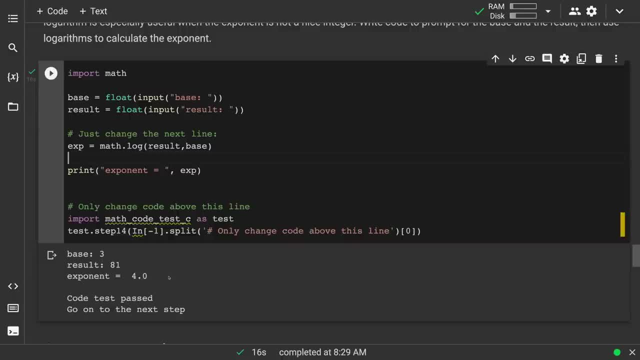 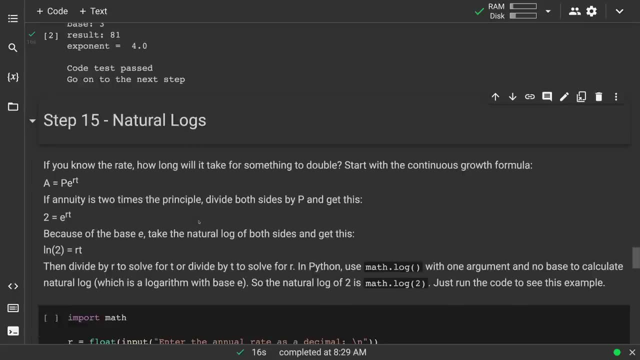 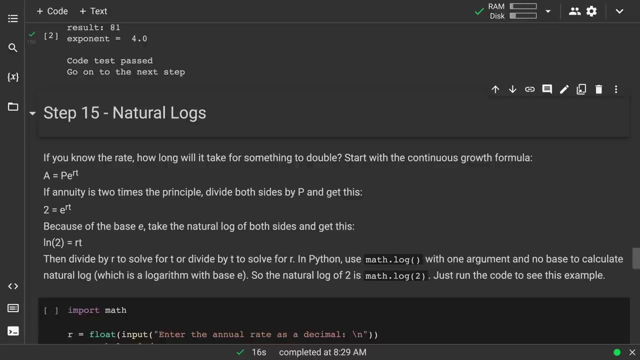 But this is useful. Three, to what exponent gets you like 80? Or gets you 85?, You know, when it becomes some weird decimal. All right, so natural logs. And we talked about E. So this is the. this is another use of the logarithm. So 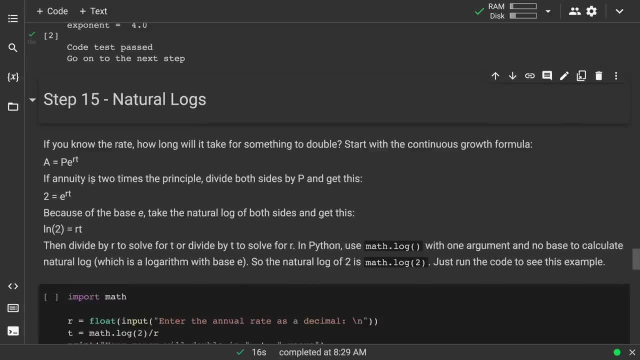 E. And just to recap, if you have this formula, annuity equals PE to the RT. There we go. So supposing I want to know how long it will take for something to double, And you'll see the logarithm connection here. So you know, whenever I start out with P, the annuity needs to be double. So 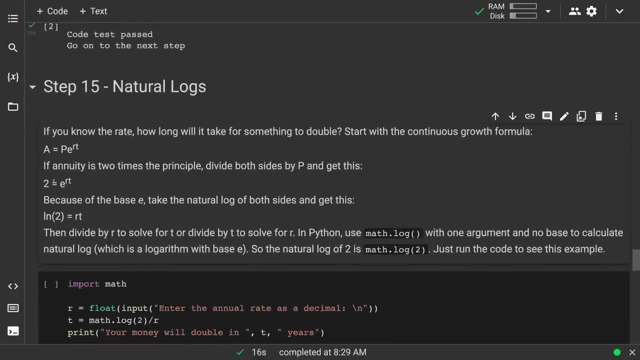 if the annuity is double, then the annuity needs to be double. So if the annuity is double, whatever P is and annuity is twice, then I could cancel it out. You know annuity would be 2P. 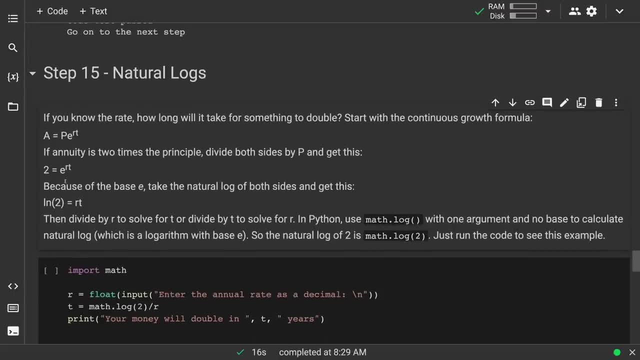 So it simplifies to this. And then now one of the many situations. I want to know the exponent. Well, I have base E, So math terms, I would say natural log. I'd do the natural log of both sides. 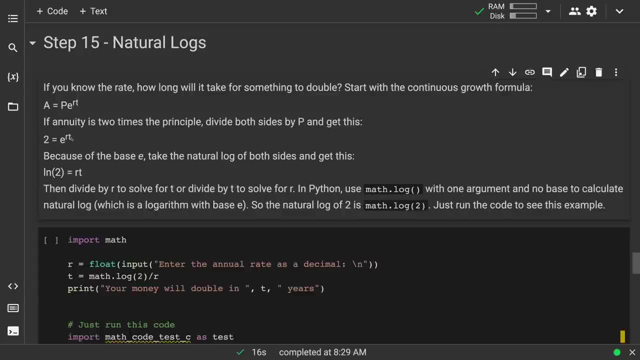 the natural log of two on the left and the natural log of E to the RT. And remember then that cancels The natural log of E to the RT because that says E. the natural log says E to. what exponent gets me this? 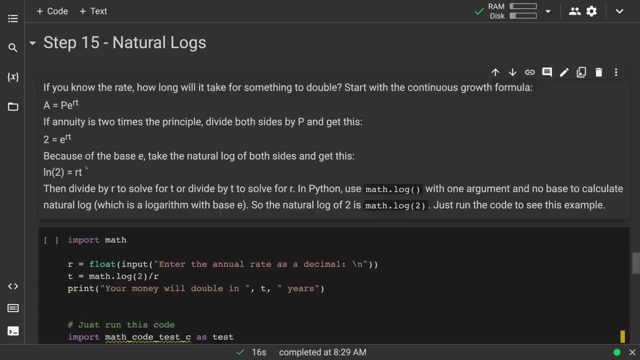 So E to what exponent gets me E to the RT? Well, it's obviously RT. So now we're in this situation. We know that. take the natural log of both sides. Now we're in this situation And I get natural log of two- Good thing, I have a calculator to do this- And then 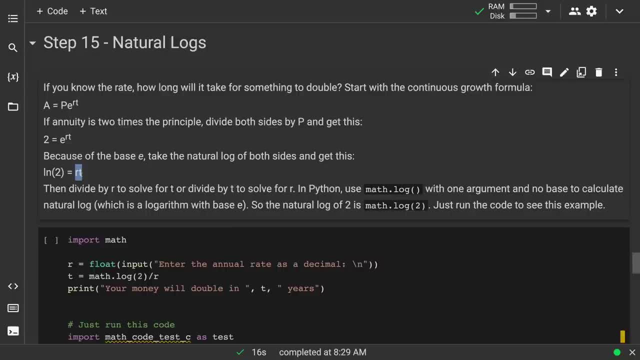 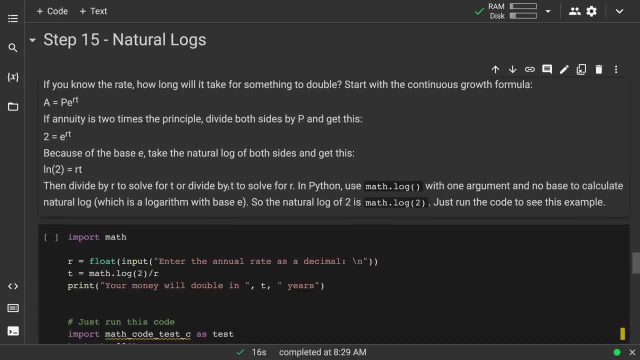 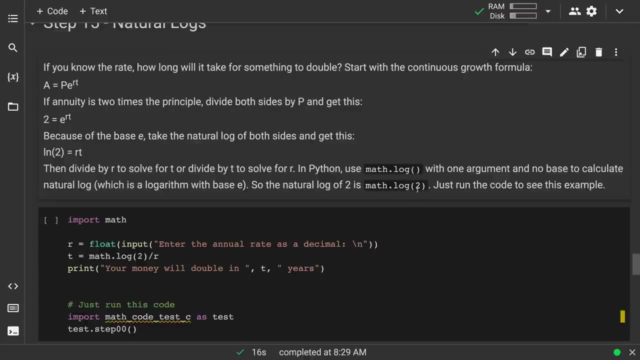 if I want to know how long it takes to double, if I know the rate, then I would just divide by the rate And then my answer is time. So in doing that math dot log and you see no other argument necessary If I don't put the argument. 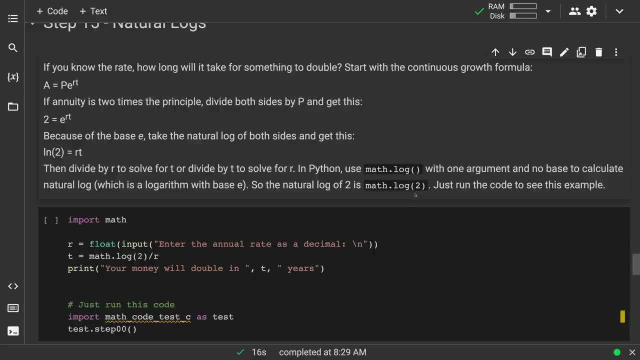 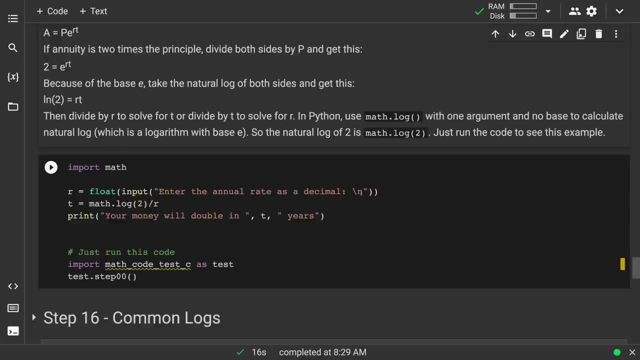 of as far as what base it is. it takes it as base E, natural log. So there we go, And in this one R input the rate as a decimal. And for this one I just put the end, just it's this seem like a long sentence? So the input comes in. 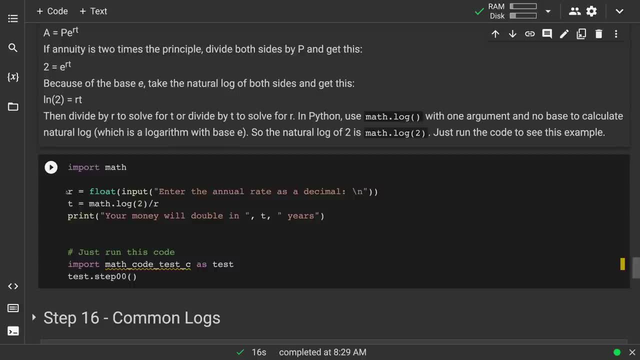 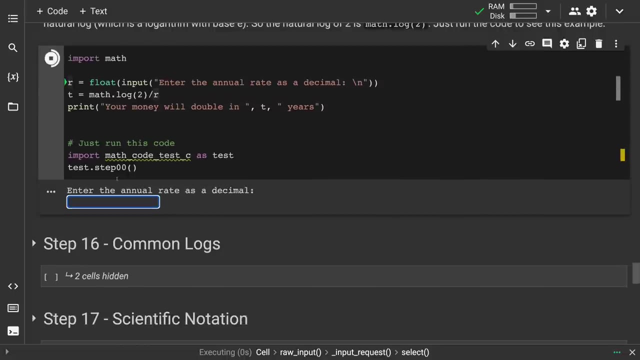 as a new line on a new line And once the person input the rate, there we go. It's just math dot log of two divided by R is time And we'll print out. it will double in T years. This is pretty useful, So you can run this Now, this one, remember? you just needed to run it. 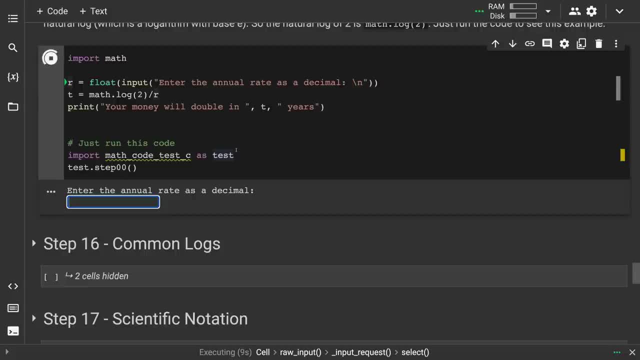 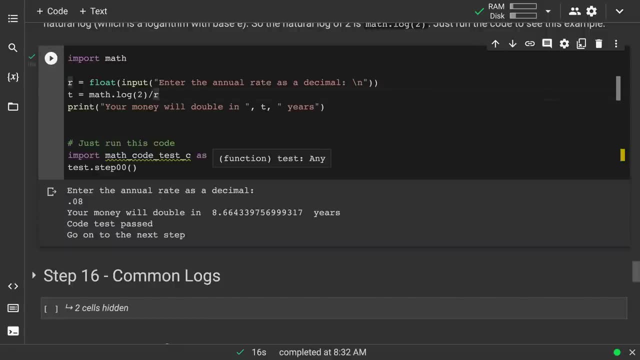 And put the rate. So if let's say, I have some investment growing at 8% and it will double in 8.66 years, So some of the you know you might say, all right, my investment's growing at 8% And we can even round this down to eight and a half. 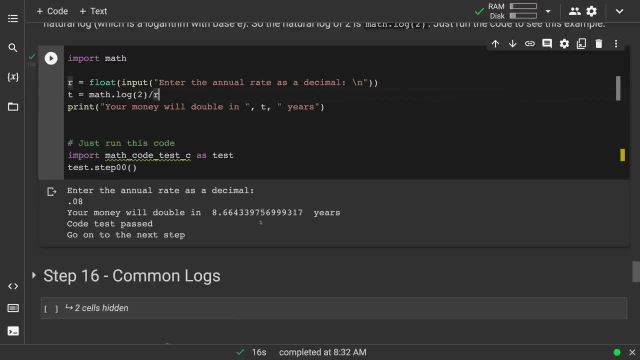 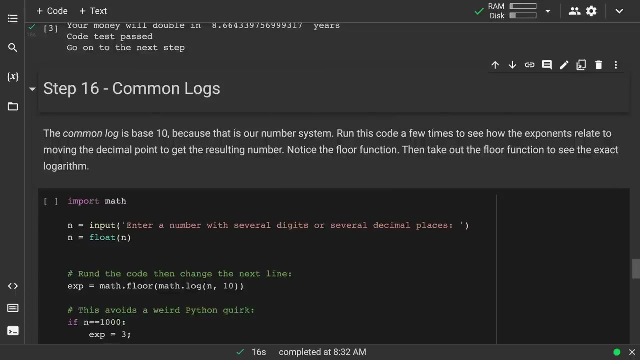 And you can do things in your head. Okay, well, eight and a half years it'll double. 17 years it'll double. from that you know, etc. And you know you could use this to estimate some outcomes. All right, common logs. So if I have base 10, it's the common log. If you were, 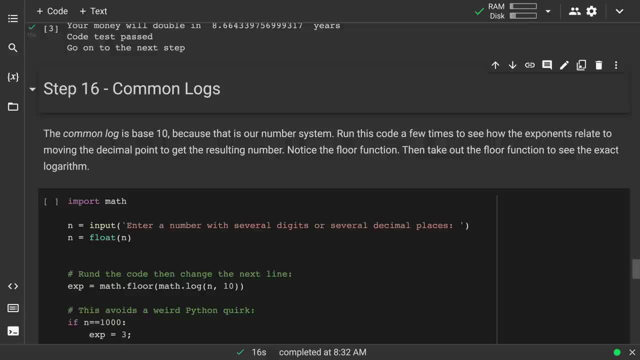 writing this in math notation, you would just, you could just say: log. So with, without the little number, because then you know, if you don't put the little number, then we'll take it as base 10, because that's our number system, the common log. 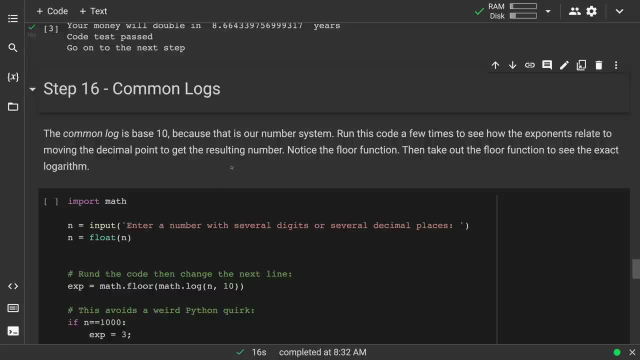 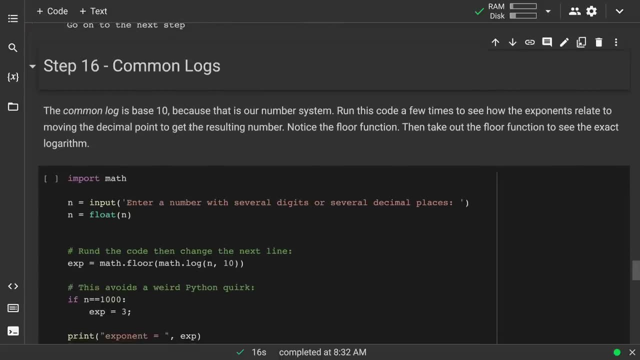 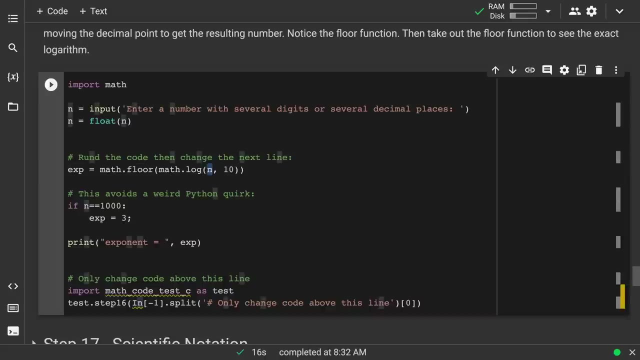 So this is what we're going to be using when we want to have. you know how many decimal places do I have? we're using things for scientific notation. So in the code, you see, we'll just do mathlog n and then base 10.. So you see, if I don't say the base it's e, but 10, even though 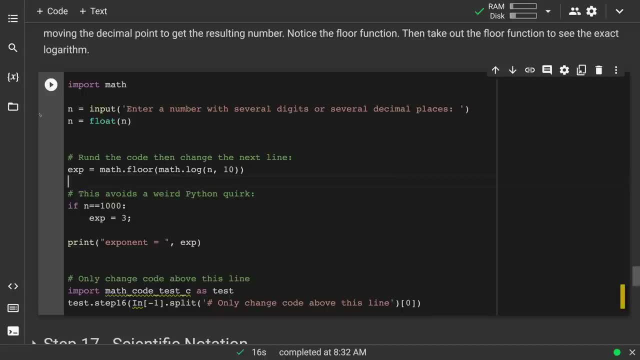 it's common. I do have to say the base. There we go. So if we have this and our number with several digits or several decimal places- and this one I just separated into two lines to show you can do that also, take the input. 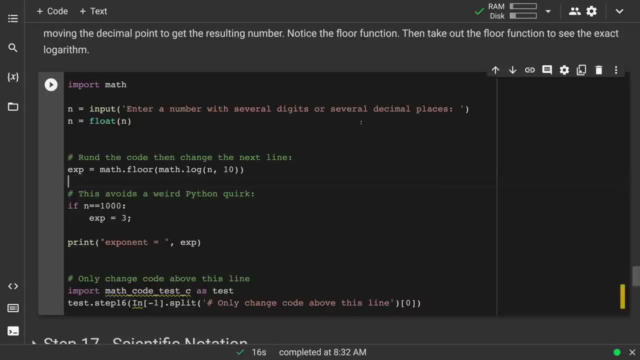 you know, cast it as n. The other reason to put this into two lines is you might notice this vertical line over here, Maybe even before writing Python. you know you might have the sense of. you know you only want the lines to be the same. But if you want the lines to be the same, you. 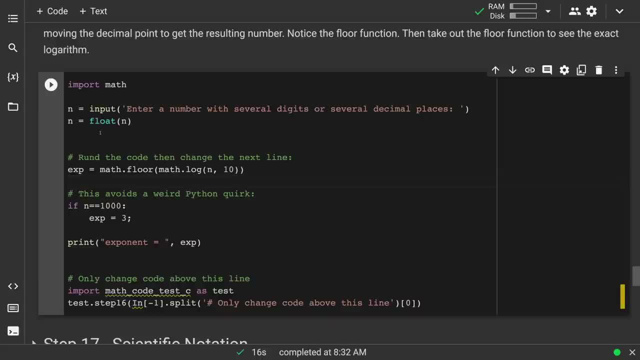 don't want to have to scroll over, But Python really makes that a design decision. If I continued beyond this line it would still work. it wouldn't just cut off that code, But just as a convention for writing Python code we usually make it. I think it's like 80 characters brings it over to. 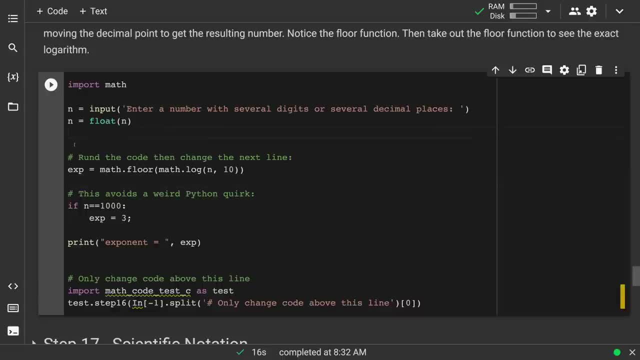 that line. So there we go, I have this one, And then I didn't want to go further on that line, So I just made it a separate line, casting that as a float. Okay, so now, all right, now we have the round, the code, So this one, we have math dot floor, So I'm going. 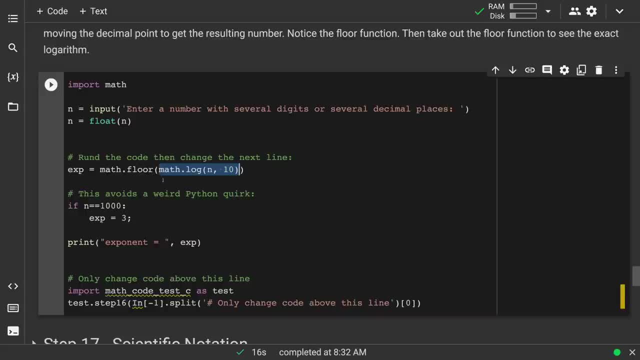 to take the log of that. But I'm not going to round, But instead of run, I'm just taking the floor of this Because I don't want the decimals, I don't, I don't want to potentially round it up And I will just, you know, drop the decimals math. 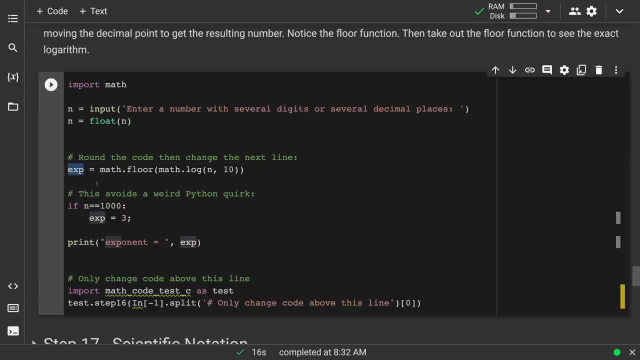 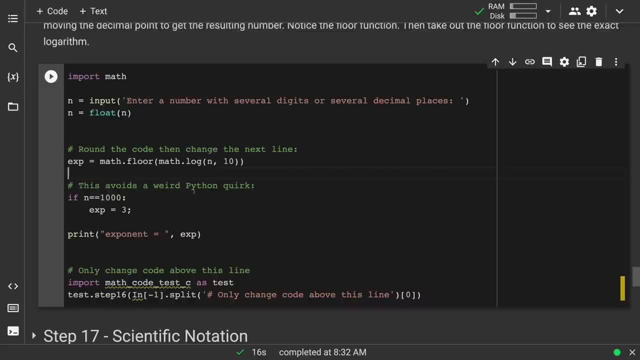 dot floor. That's going to give me my exponent And that's actually what, what we really want. And this is a weird Python quirk. When the exponents exactly three, it sometimes doesn't give you the answer you want. I don't know, it's just weird Python quirk. So just bonus insight here after: 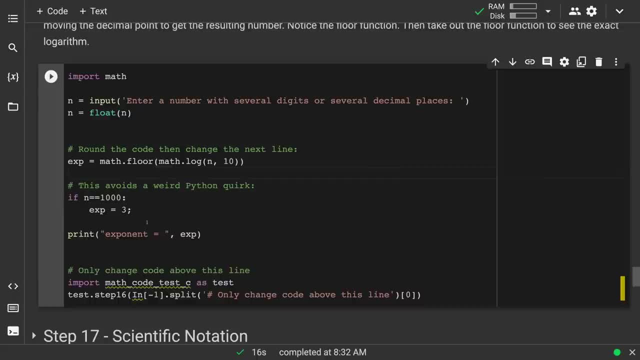 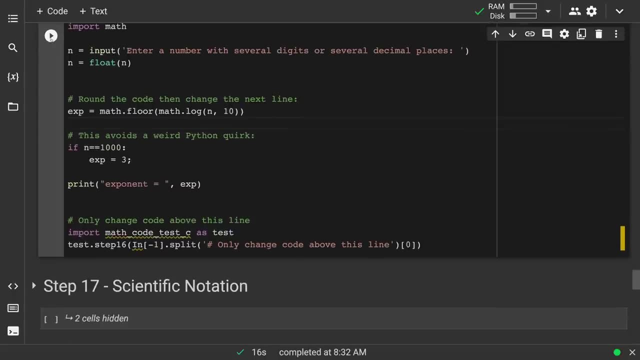 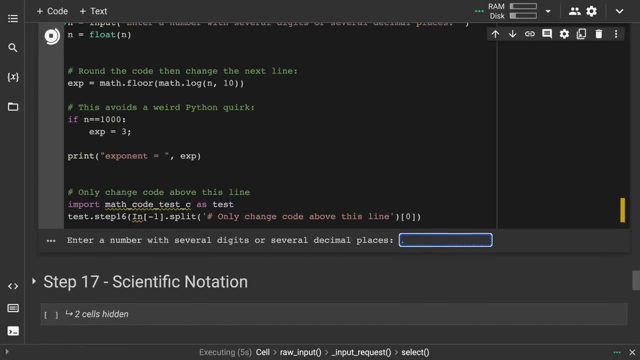 doing this enough times. I just added this little if statement here: All right, And we're going to print the exponent. So when we run it we go several digits. So if I have point, you know 0005.. All right, and 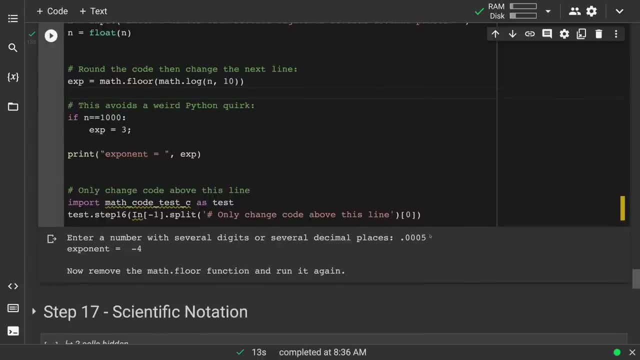 we can get the exponent, And the exponent is negative four. Yep, There we go. And if we remove the math dot four function, then it will just give us- it'll be you know, negative four point- something else, And we'll just do that. 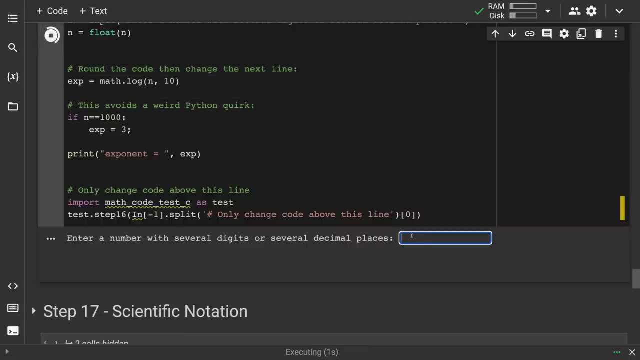 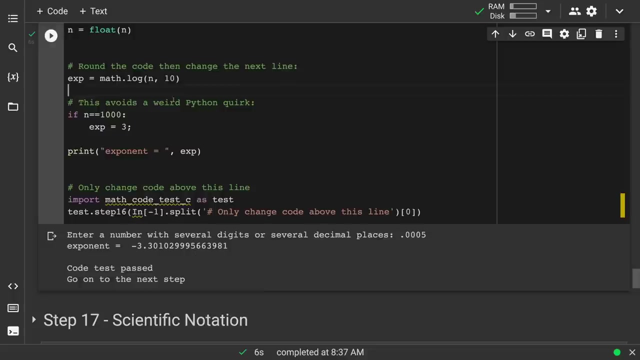 There we go, So you can see, and I'll just to compare, I'll do the same number: .0005.. All right, And that's it Now. notice in positive numbers it would be four point something or three, if this was positive. three point something. 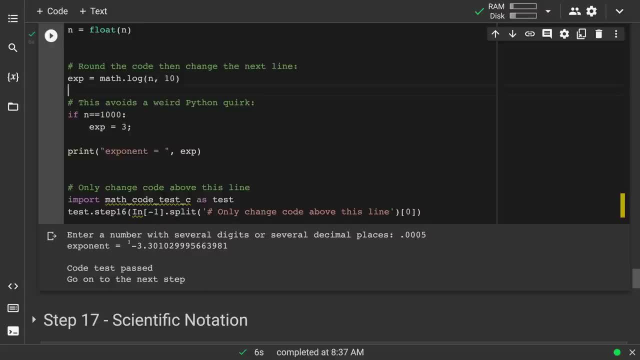 and it would drop the decimals. it'd be down to three. But with negative numbers the floor from negative three point something the floor of that is negative four. So just interesting insight. And again, you're watching this video because if you've gone through the 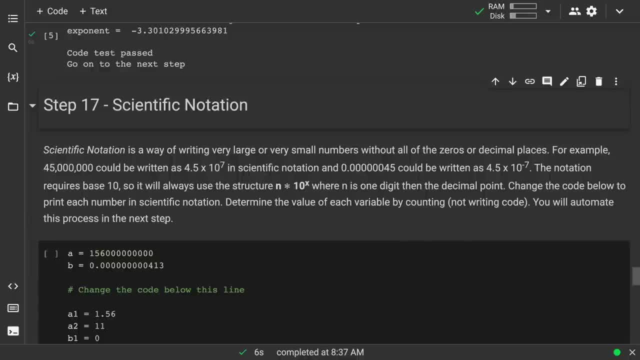 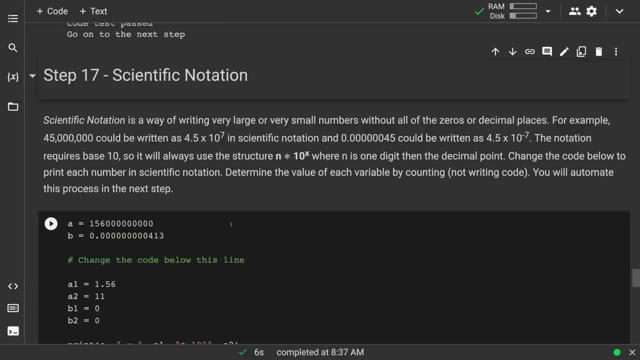 foundational math three and maybe you're stuck on something or you want some other insight into some of these. so hopefully you know this helps. All right now, all that you know, we can use these logs, the logarithms you know. 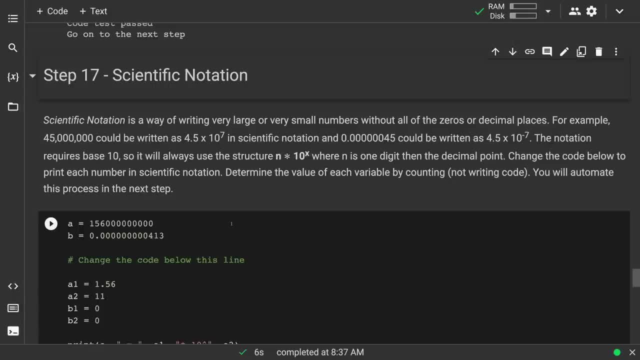 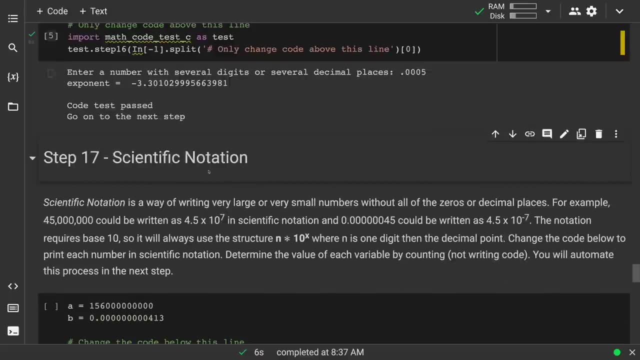 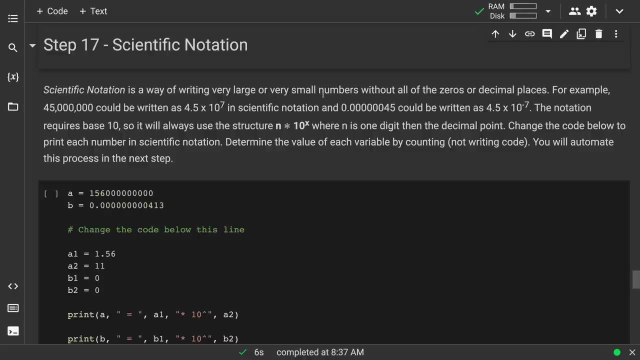 how long to take something to double. you know things like this number of decimal places. and notice, I called that exp for exponent because well, first of all, that's what we're asking for in the logarithm, but also that leads to scientific notation. 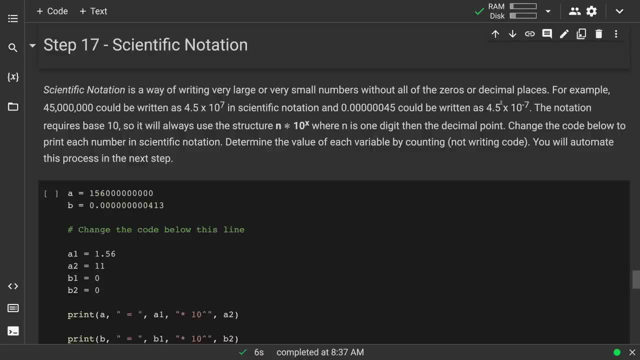 You know how can I write very big numbers or very small numbers without all those zeros? So if I had like 45 million, oh, but I can write that as four point, five times 10 to the seventh, or point zero, zero, zero. all these. 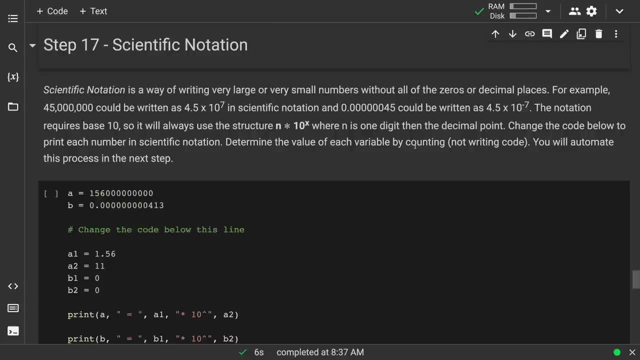 could be four point five times 10 to the negative seventh. And there we go. So it's always n times 10 to an exponent, and n is always one digit than the decimal. So that's what we want, you know, because four point five. 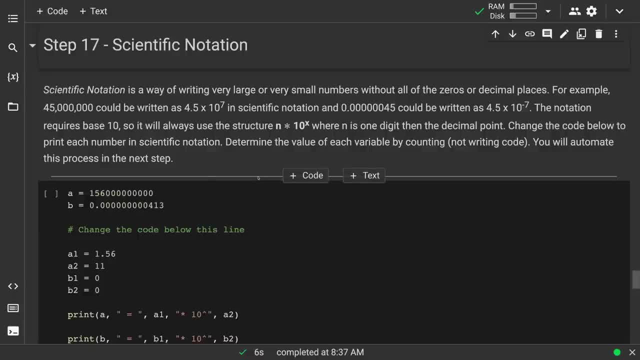 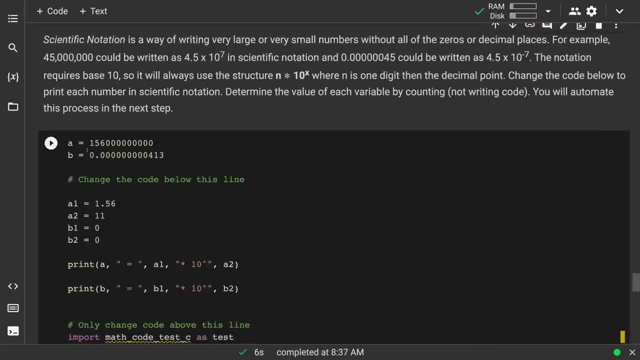 that's. I want that one digit than the decimal. That's the true scientific notation. Now this is just changing. you know this one here we're not actually writing code. This is determine the value by, just by counting. I just wanted you know, just to see. 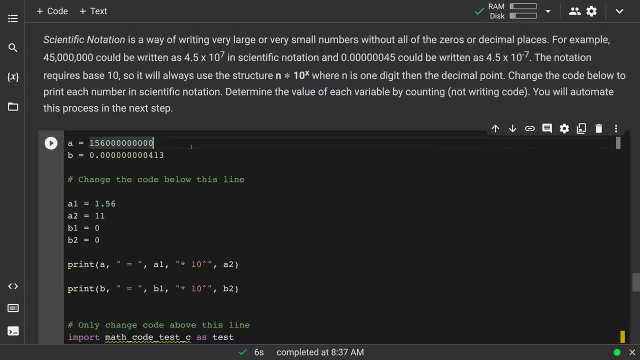 You know, as we count. so, how many decimal places, how many places One, two, three, four, five, six, seven, eight, nine, 10,, 11, because it has to be, you know, 12,, 13.. 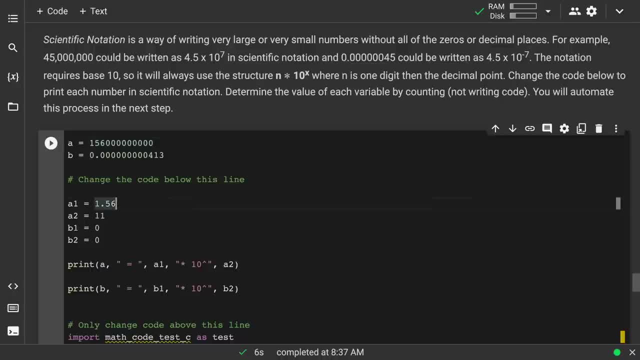 down to this. so that's why we have a 1 is 1.56. that's where the decimal would go, and a 2 would be 11, and then we're gonna print that out, a that there is a 1 times 10 to a 2, so then we'll do this for here. so the decimal point would be: 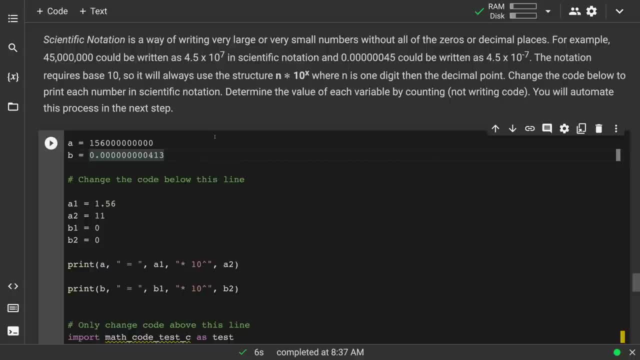 there. so then it's yeah. so then we would move it 1, 2, 3, 4, 5, 6, 7, 8, 9, 10, so it would be 4.13 and we have to move it in the negative direction, so it'd be to the. 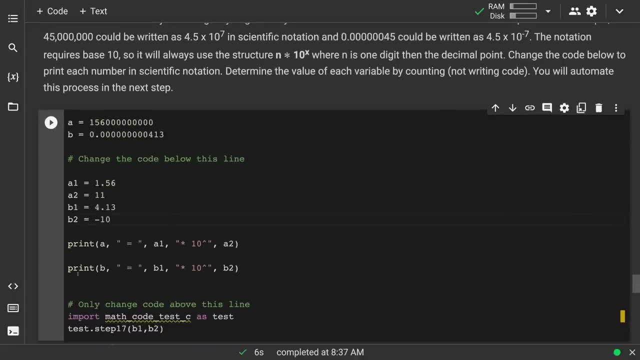 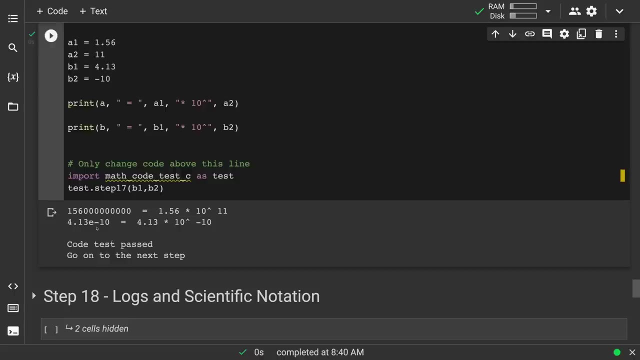 negative 10, and so then that would print you: the is 4.13 times 10 to the negative 10. there we go and we run it. there we go. now this one works, displays nicely this one. how we want to display it here is nice, but Python automatically and this is: 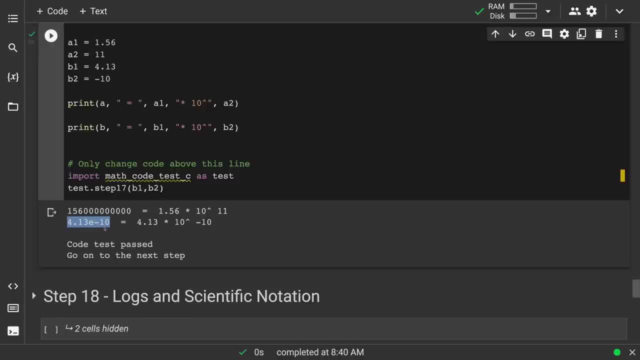 fine, and then we're gonna run another one. so we're gonna run this and we're gonna this one. how we want to display it here is nice, but Python automatically and this is fine, you know, you go on to the next step, But Python automatically converted this one. 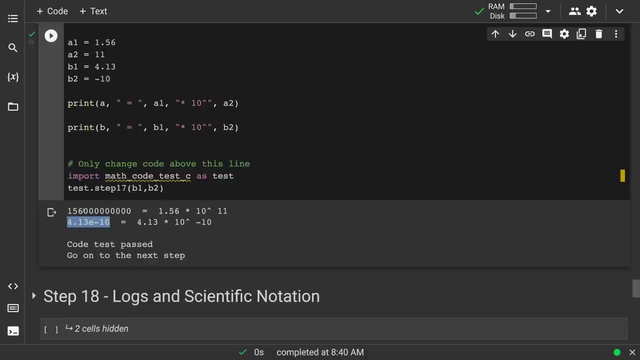 A positive 11th power- fine, It didn't see a reason to change that- But negative 10, so that's the Python notation: 4.13e, negative 10.. So, and this is not the same e, this is just indicating exponent. 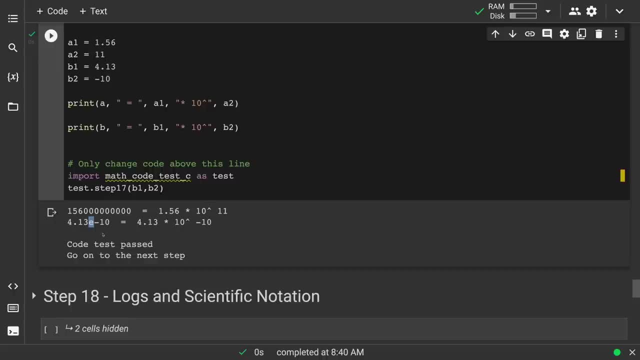 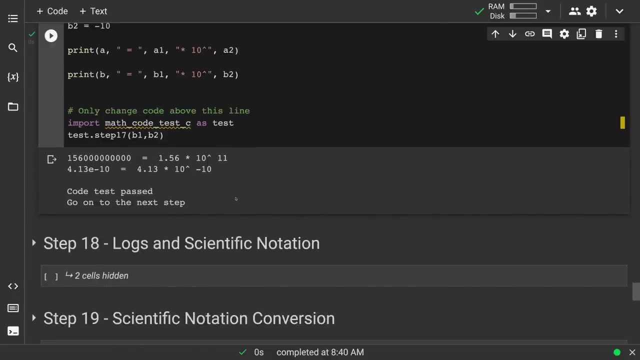 So times 10 to the negative 10.. So there we go. So in this you know, hopefully also again if you're watching this it's, you know, illustrating like why there's some of these quirks in Python. 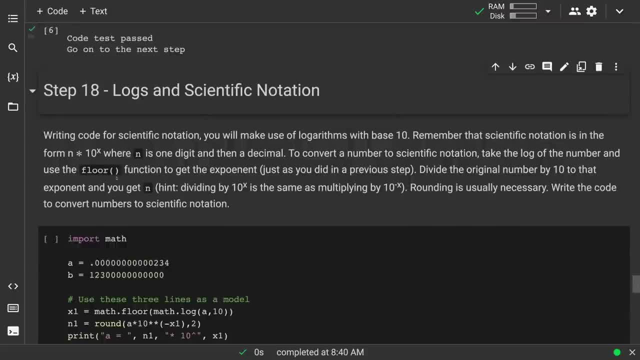 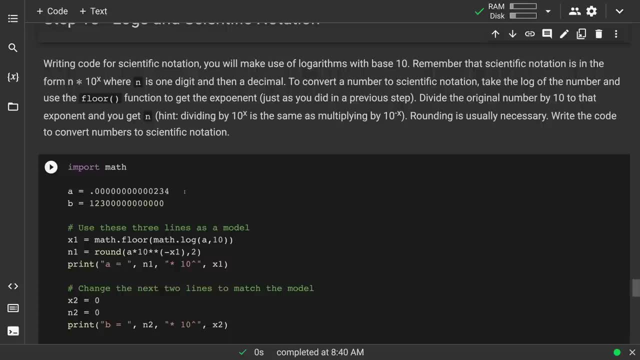 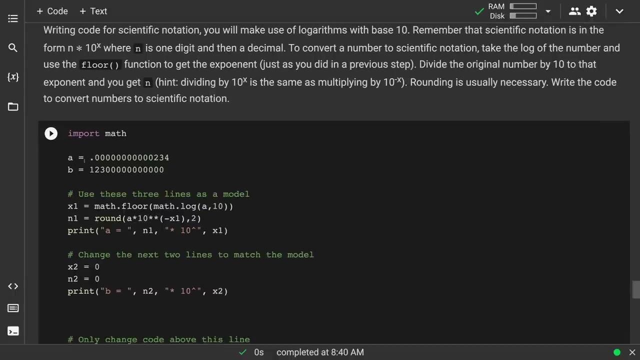 All right, so we can use these logs for scientific notation, Because if I want, you know if I want to convert this to scientific notation in an easy way, so what do I do? So I did this for a putting together the things we did in the last two exercises. 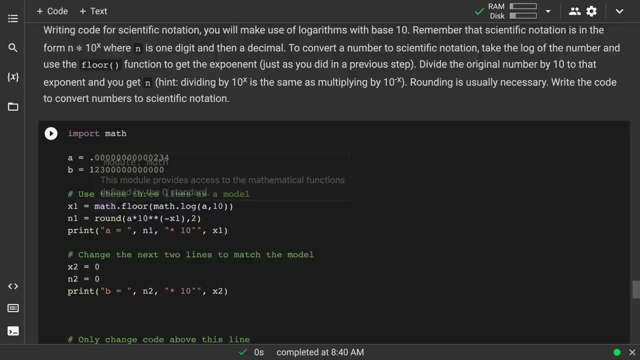 So for a, I'm going to do the floor of the log of a base 10.. There we go, And now I'm going to round it. So so it was a. I called it x1 for exponent one, And so, if I have this a times 10 to the negative x1,. 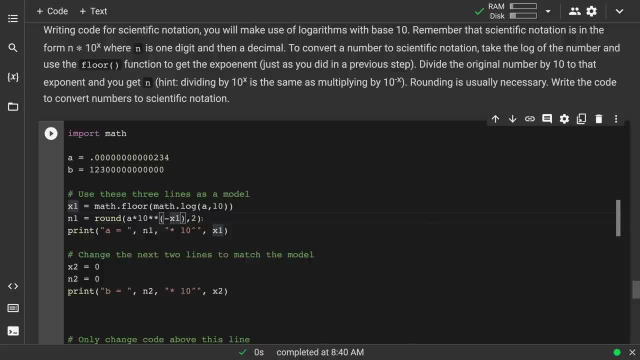 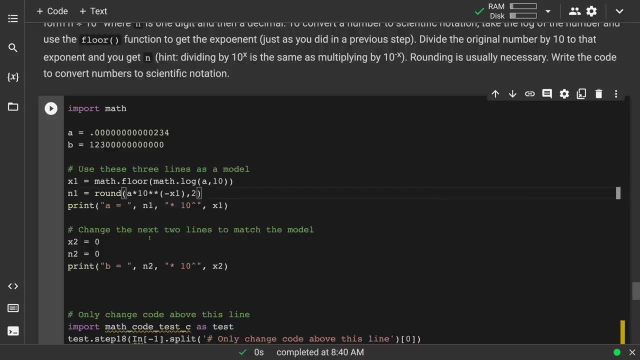 and it rounds it to two decimal places. So if that's the, if that's the log, then I'm going to multiply this times 10 to the negative x1, and it's going to print this out. So I'll just show you the code. 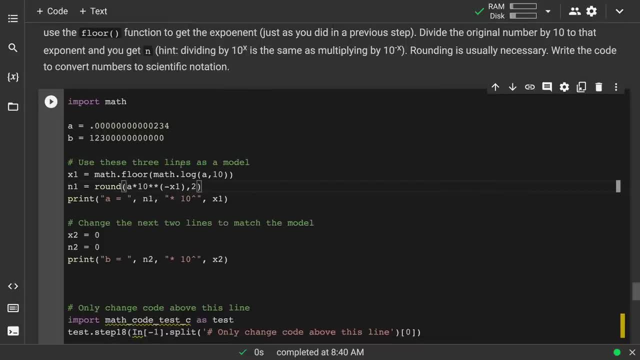 and then we'll run it and you'll see. So now, using that as a model, what I want? x2, and I want to show you that this actually works for positive or negative exponents. Yeah, So, if we have so, but this one. 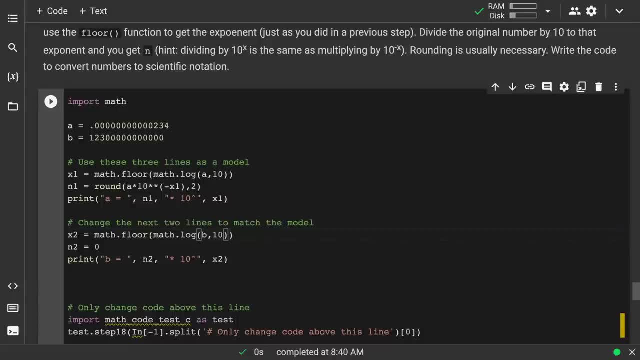 I want this for b, so take the log of b, base 10 and the floor of that, And if I have this then I'm going to round that. So I'm going to round that again, referencing b this time. 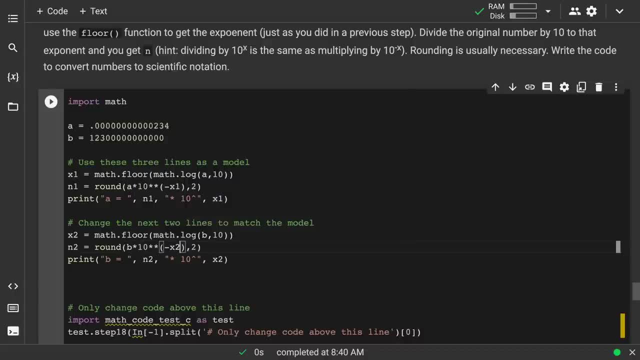 to negative, and then I'm going to round that b base 10 to the negative x2.. There we go. So it's what exponent got me there. but then when I take that, then that will divide it out. That's why it's the, that's why it becomes a negative exponent. 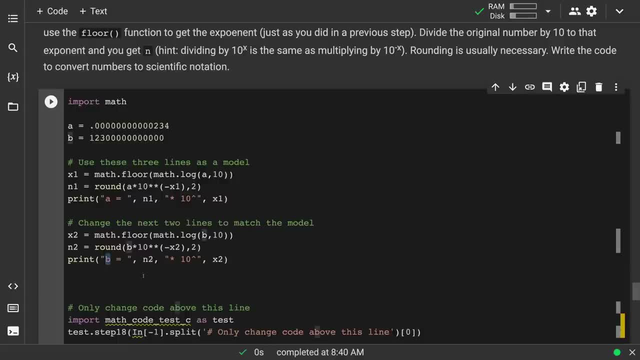 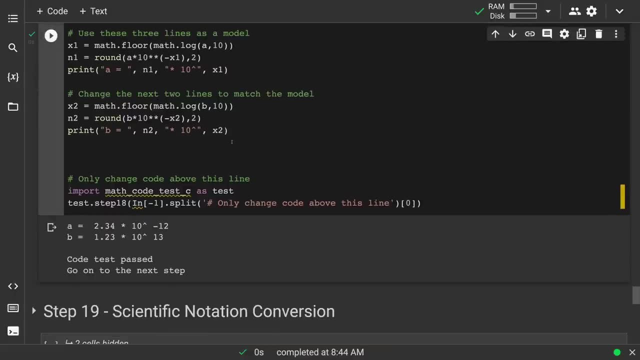 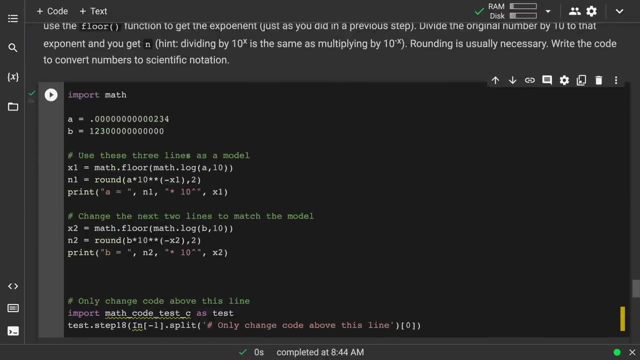 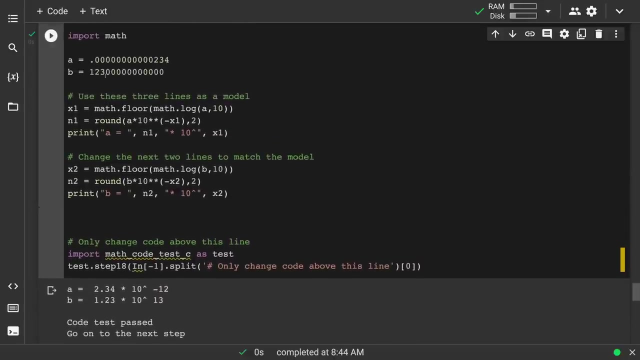 because I want to divide it out to get that early number there. All right, So if we run this and this just took those, So you see we get a is 2.34 times 10 to the negative 12, and b is 1.23 times 10 to the 13th. 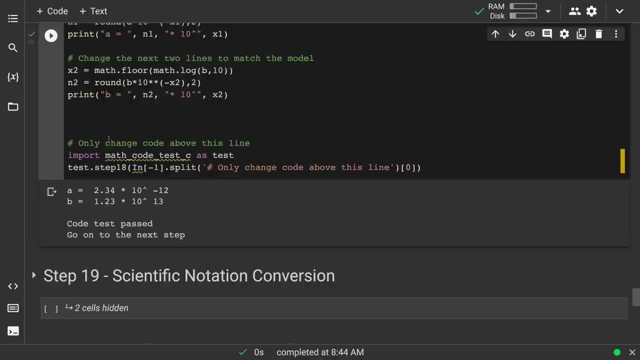 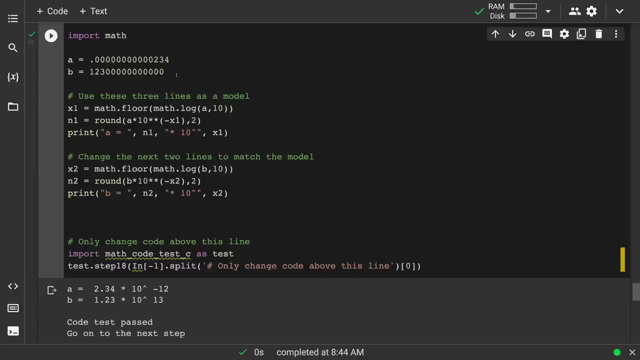 So pretty cool how you could just take this and whether I wanted to show you that whether it be a decimal, so a negative exponent, or a huge number with a positive exponent, either way this works. Take the log base 10, and the floor of that. 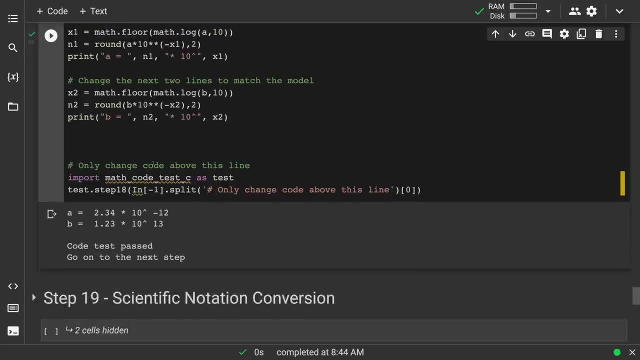 and that to the negative exponent. that's how we get n1, then we're then multiplying it by that and we can display it. So this way, now you have it, You can have a code to convert anything to scientific notation. 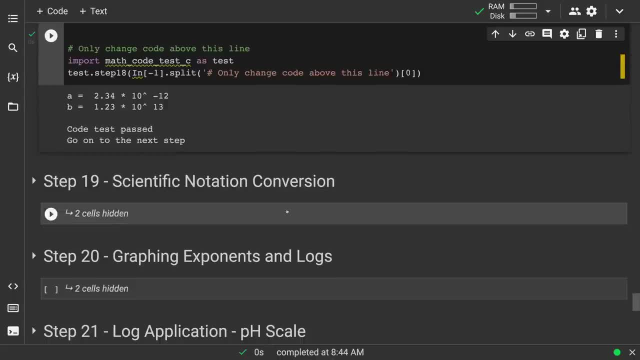 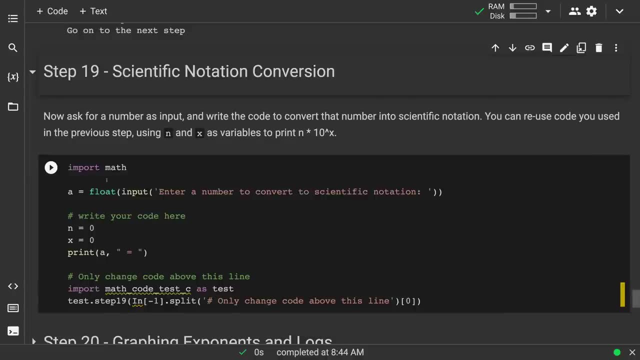 Pretty cool, And that's what we get into step 19.. There we go Now, this one, very similar to what we were doing before, And we're just added one more thing of entering a number to convert to scientific notation. So see, this is where you can make it as your calculator to convert. 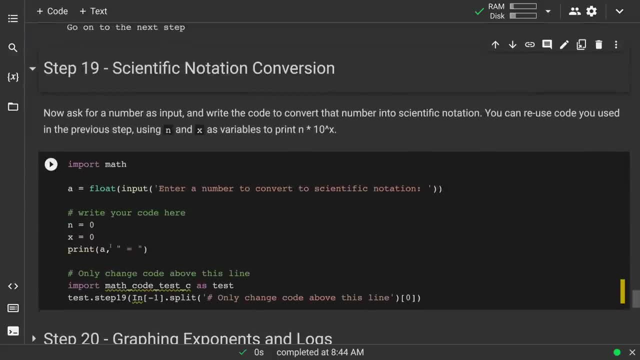 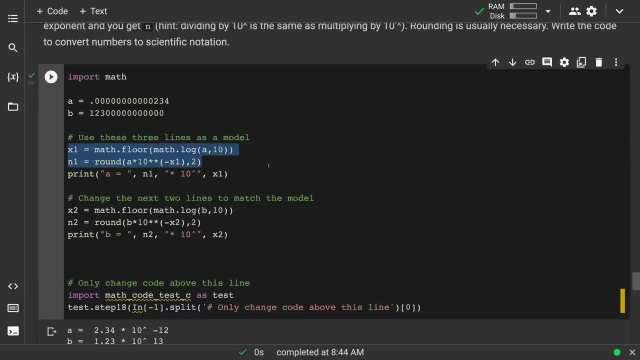 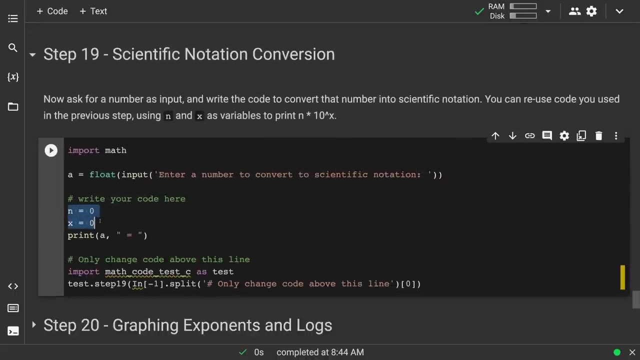 but you can also convert it to a number Convert, because I'll just take this and it works either way. I'll copy this code that we had from before and paste it here, but I don't need the number ones, because I'm only doing one thing. 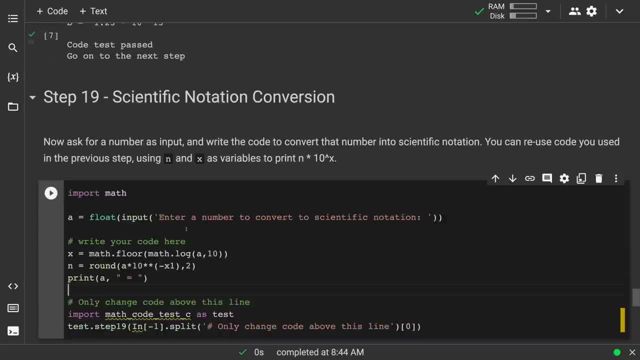 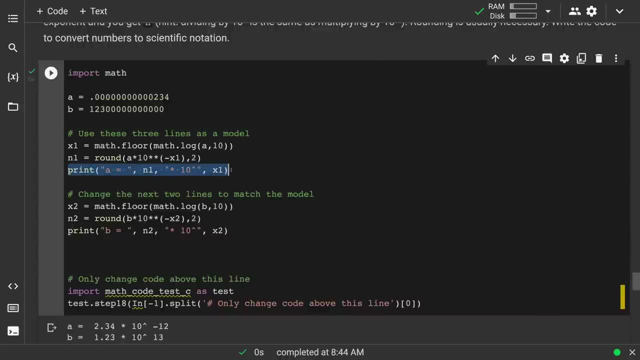 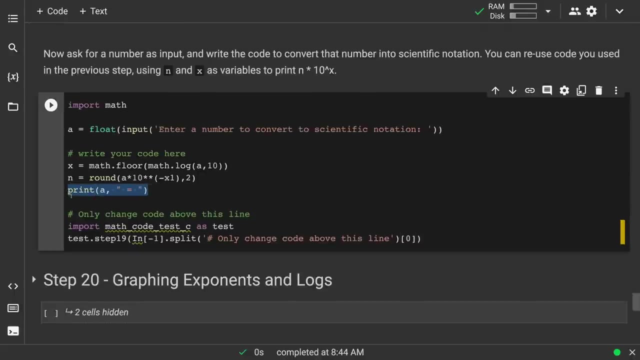 And in that case, if we wanted to print- you see, I even left this- That's what we want to print, So we can reuse this. And this is the key with copying and reusing code, You can do it, Just be aware to notice these little things. 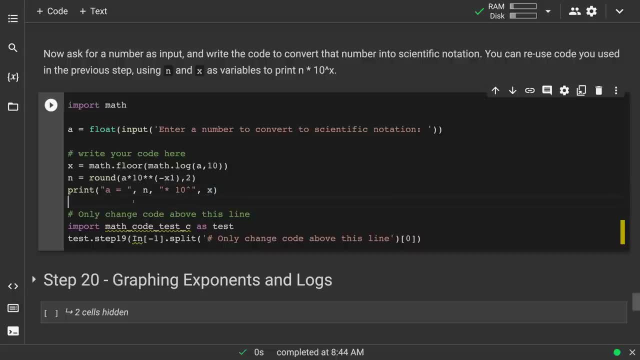 If you just copy and paste something, there might be little subtle things that don't line up. You know, just copying, pasting, no good, You have to understand the code well enough to know these little things that you need to change. 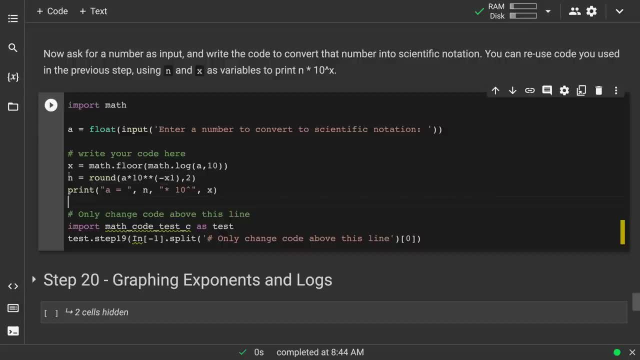 Oh, okay, I needed to delete the ones here all around And you know, copy and paste with the follow-up editing. now that works And see what you can do is now you have this as a standalone, you know input. 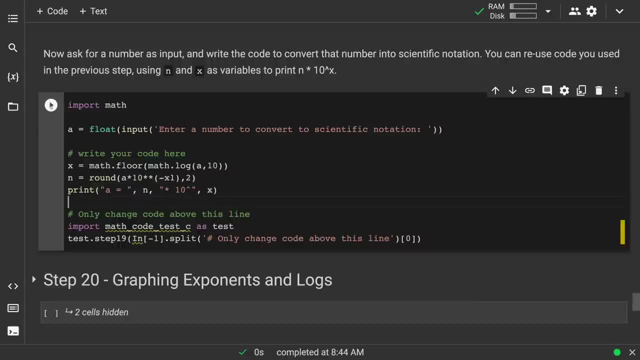 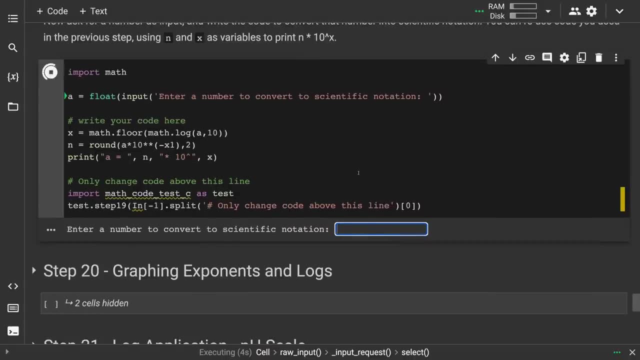 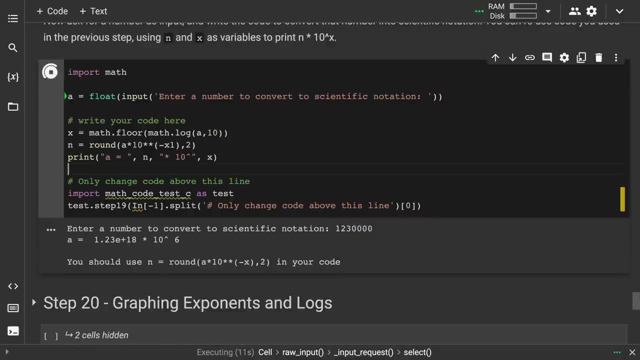 You didn't have to like define the variables in the code here And there you go, Enter in whatever number, All right. So one, two, three, There we go. There we go. One, two, three. Oh, that's very weird. 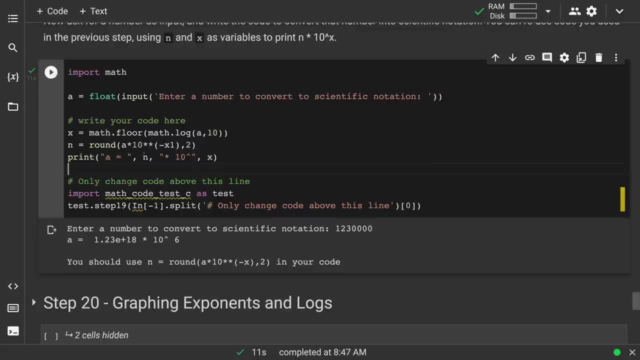 One, two, three, I got to 1.23.. Ah, look at this, It see. as I was mentioning it, I didn't delete the one there And that variable was still in memory for that little bit, so it gave me this, you know exponent that I was not expecting. 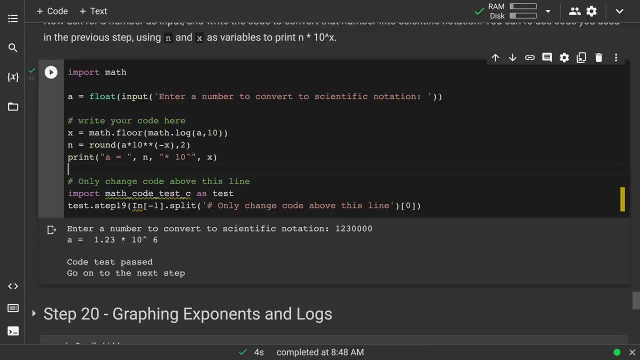 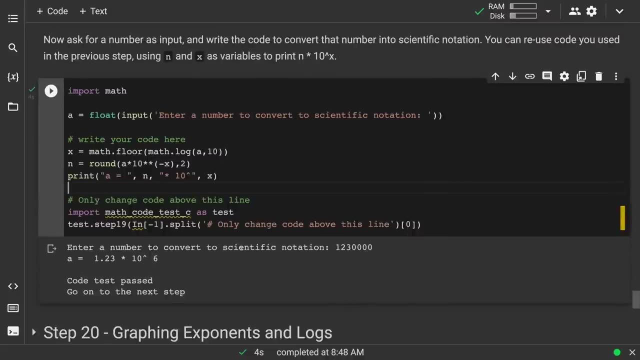 One, two, three. There we go. All right, Pretty good. So anything that you have now- now we have this standalone code, And then later on, what we're going to do is- and then maybe I'll use this as an example- 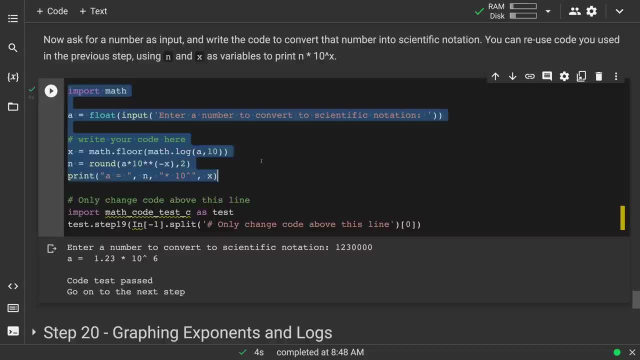 is, we can put all of this code within one function, And so then now you can just define a function that will convert to scientific notation And all this code is within that function, And we can take that and then that function we can use wherever. 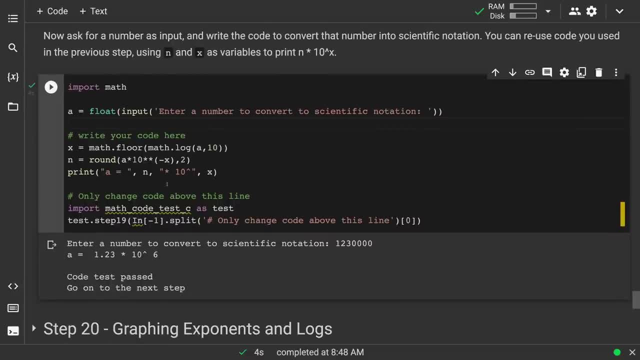 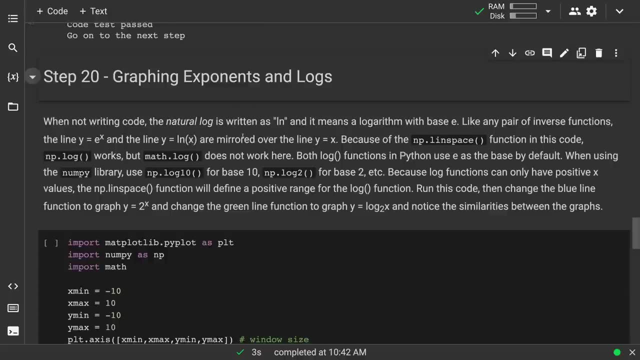 All right, So let's go on to the next one. Now we'll get to graphing exponents and logarithms. So just connecting with the math: natural log. is ln Putting the adjective first, Natural log, if I was just writing it on the table. 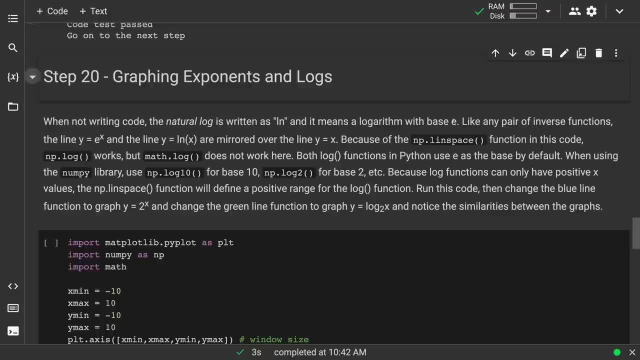 on the board it'd be ln And that would be base e, And so comparing y equals e to the x and y equals natural log of x, those two are the inverse functions and mirrored over the line y equals x. So when we see the graph, we'll see these. 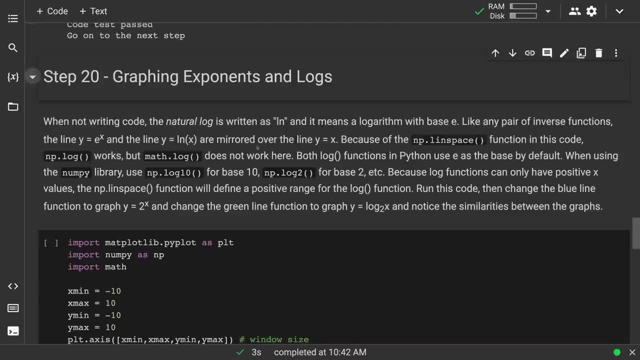 and then we'll see the line y equals x. So we were just talking about using the math library. I just want to calculate a logarithm. I'll use mathlog, But because when we graph we're using numpy and we're using the linspace function to create an array of values. 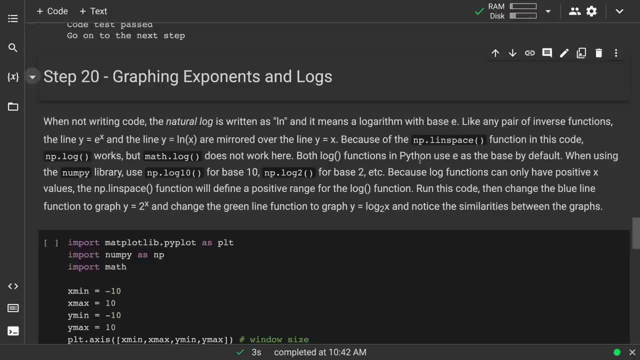 that we're going to graph, So I have to keep with numpy, which I usually import as np. So then I'll do nplog, Mathlog. as you see, if I want to do one thing, yeah, that works. If I'm using the math library, I'll use that. 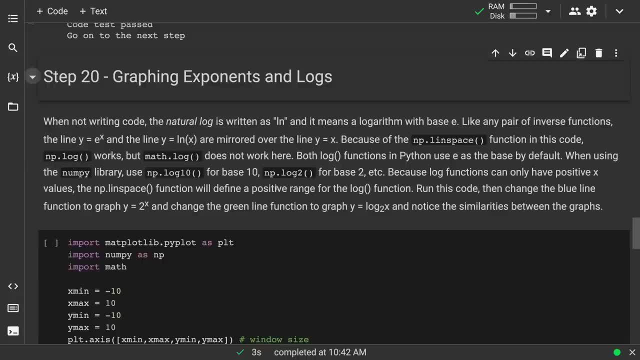 Here I'm using nplog And np has it slightly different. np has nplog10,, obviously base 10.. nplog2 for base 2. And if I just do nplog, it's going to be base e. Realistically we don't need to do every other base. 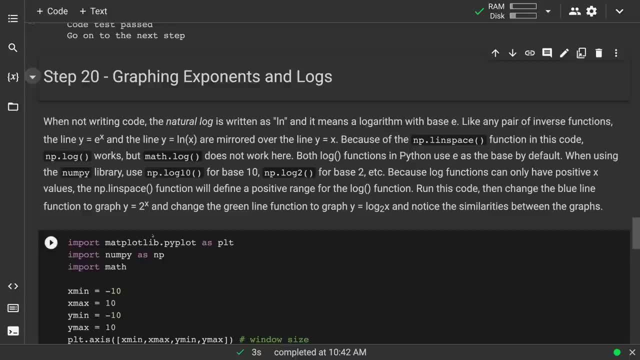 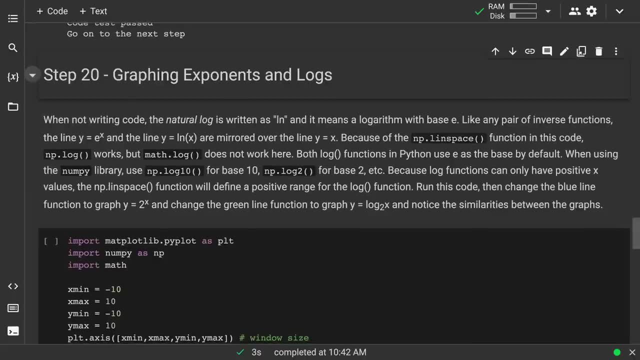 because we don't need to do every other base, Because we have the change of base formula, which I'll talk about in a second. So there we go. So we have the positive x values. Now, if I was graphing this e to the x, 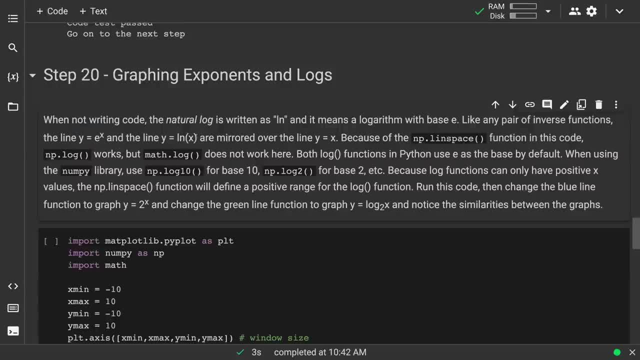 I have all my x values, whatever I want, But when I do natural log then the x value will never be 0, because, remember, they're inverses. So in this case, e to whatever exponent, the y value will never be 0. 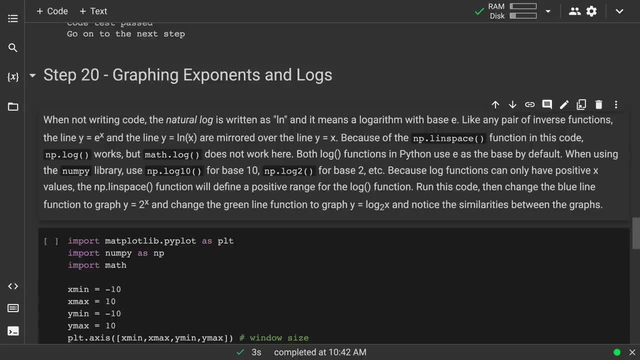 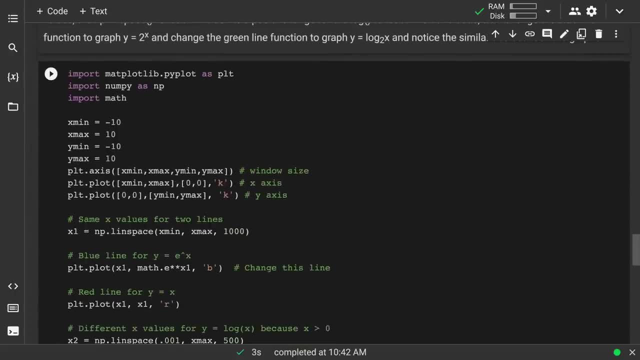 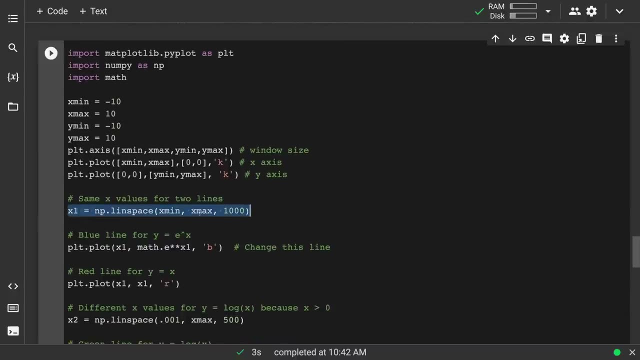 As the inverse. here, the x value will never be 0.. So when I graph this- hopefully this looks familiar from other graphing we might have done- I'm going to define this And I'll just use this minimum maximum, you know, based on here, what I did here. 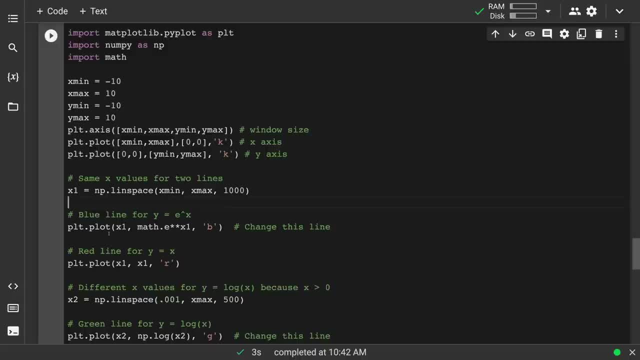 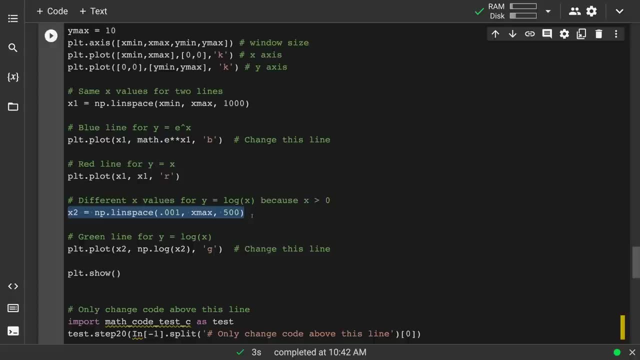 That's fine, But then when I do log I'm going to use a different linspace. I won't do 0.. I'll just pick some like really tiny number, 0.001.. And that should be enough to illustrate this point. 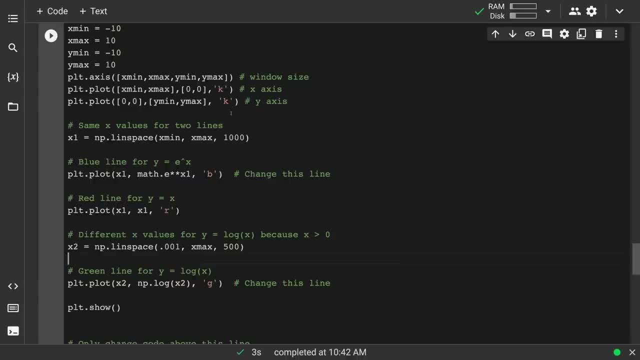 So there we go. All right, so I'm graphing these. I'll use x1 as my array of x values, And linspace goes from minimum to maximum, And then within that range I want 1,000 points. I mean for this you'll see a smooth graph. 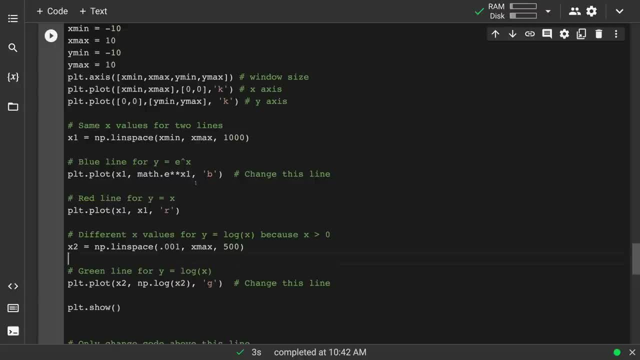 even if you don't have 1,000 points. All right, there we go. And then plot x1.. And I'll just write the y value here instead of separating it out. Mathe for my e value, And then that to that exponent. 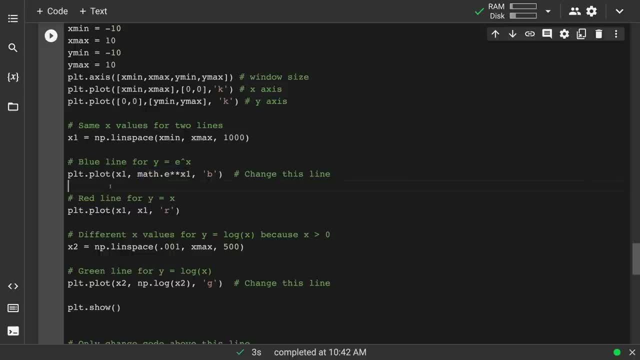 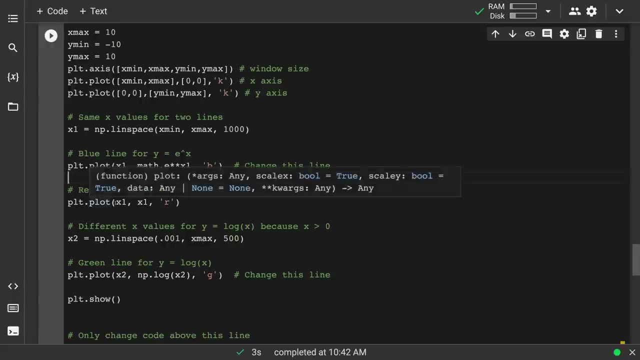 There we go, And I'll make this a blue line. So then we have the red line for y equals x, Then x1. And we see, if I have this x1. I just can put x1, x1, because it's y equals x. 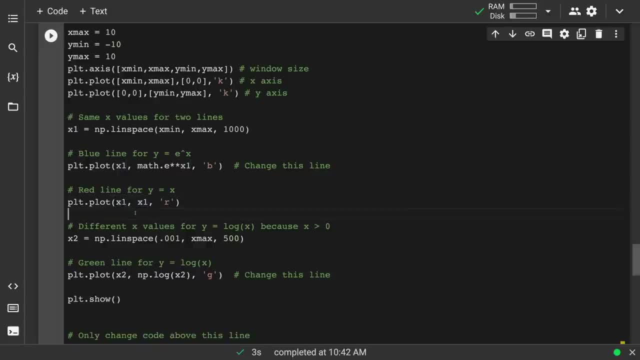 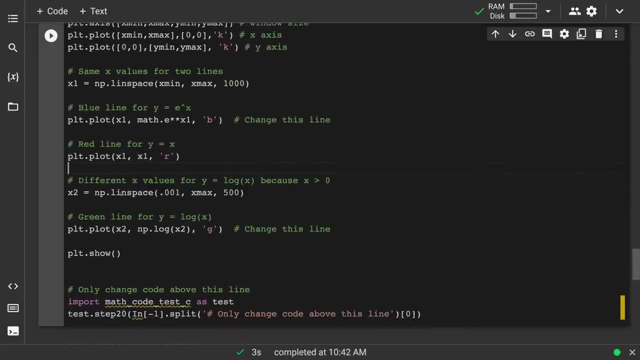 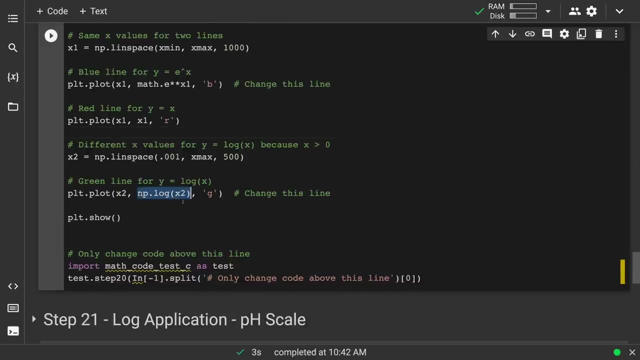 So I don't need to define a new y value. I know it's the same. And here now for my log: y equals log of x. I'll do this linspace And then nplog x2.. So there we go. 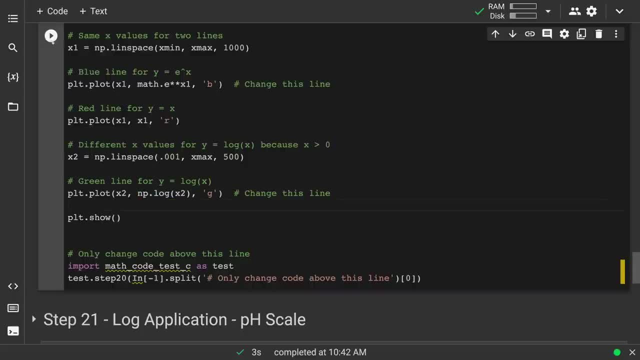 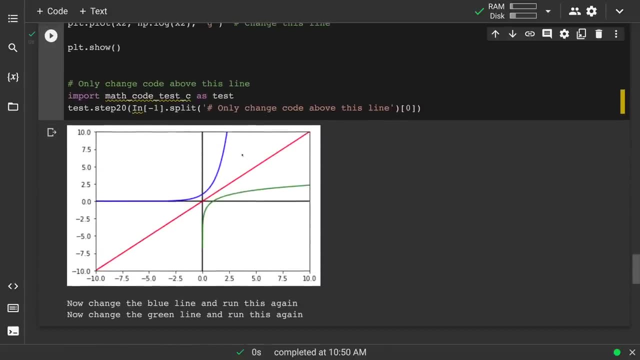 All right, So we're just going to run this and then change it. So we see this notation And there we go. So we have the blue line e to the x exponential function and graphing that green line y equals x. 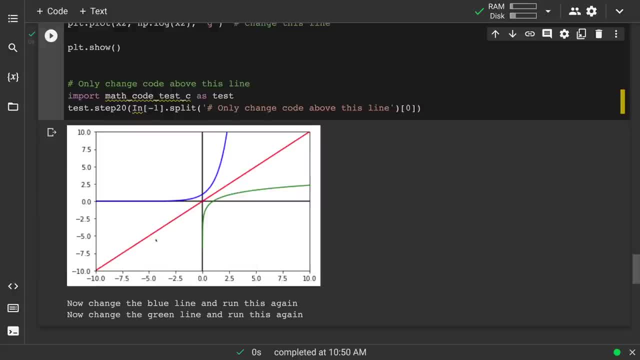 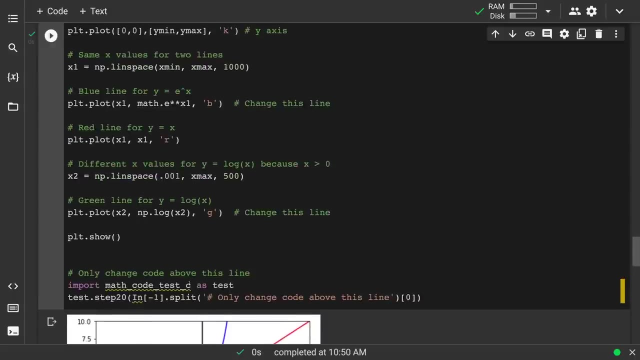 or y equals the log of x, And there we go. And this works for any inverse function. There are mirror images across the line. y equals x, But there we go. It illustrates it nicely. All right, Now change the blue line and the green line. 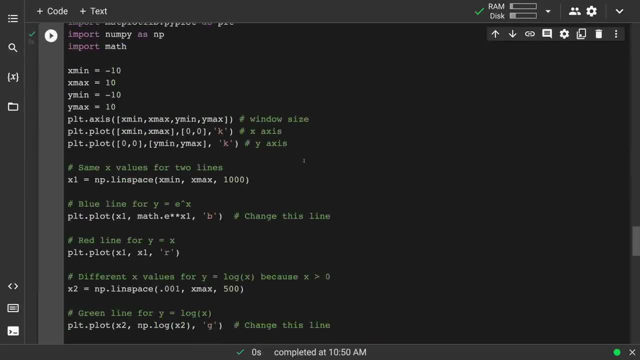 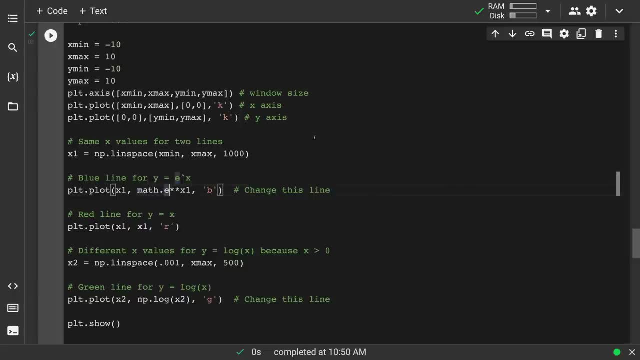 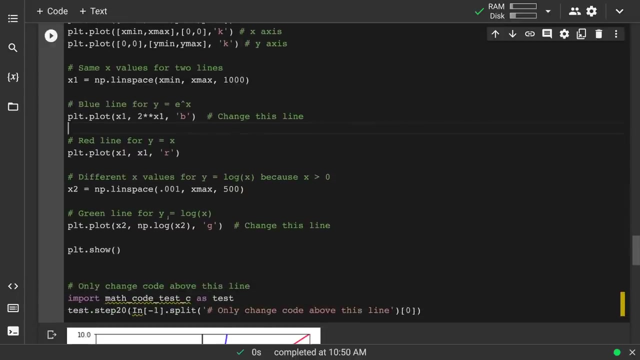 because we want to make these log base 2.. So here, instead of mathe, I'm going to make this just 2 to the x, That's fine. And this one, instead of nplog, I'll do nplog2.. 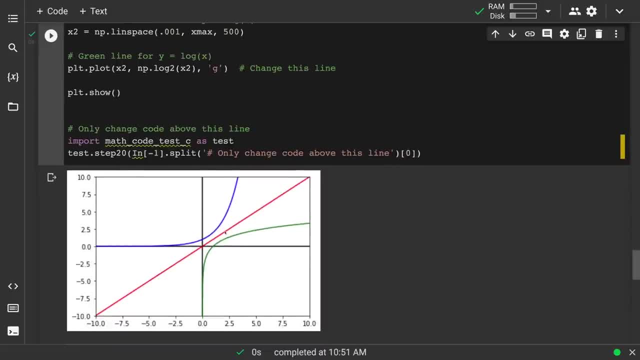 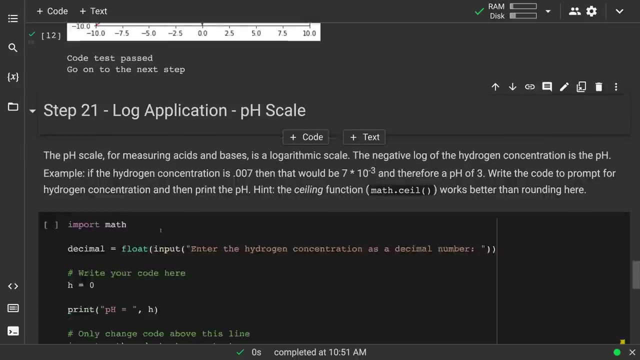 Now, we're not going to notice that much of a difference here, because I went from a base of 2.7 to a base of 2.. But there we go. That's all you need to do for this one, And I want to include some applications here. 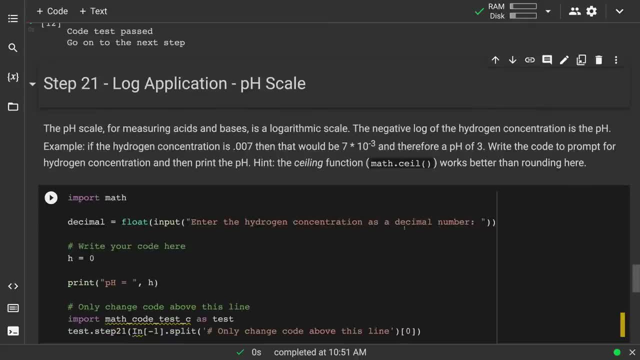 If you have the hydrogen concentration as a decimal number, that's really where the pH comes in. So proportion of hydrogen. So the way this works, it's the negative log of the hydrogen concentration. So if we have 0.007 as scientific notation, 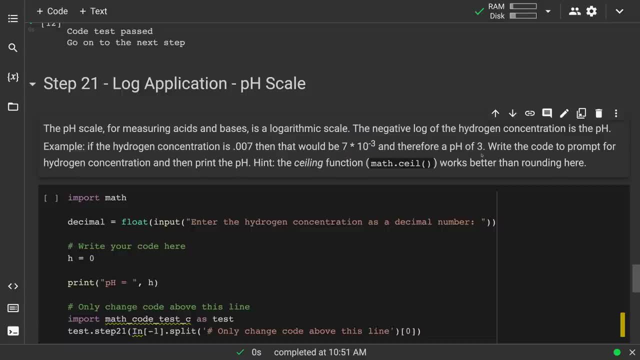 that would be 7 times 10 to the negative 3, which would be a pH of 3.. And then we subtract, And then we see that as we got more and more 0s as placeholders- a really tiny decimal number. 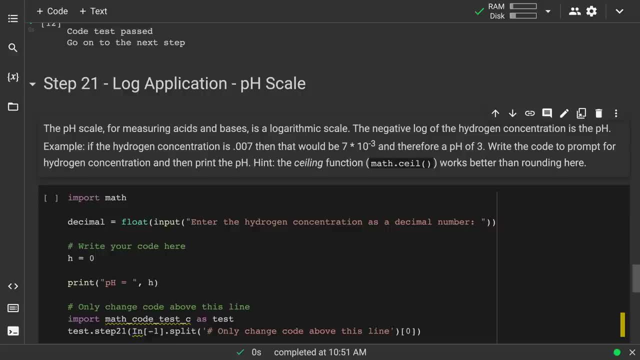 then that would be 10 to the negative: 4,, 5,, 6,, 10 to the negative: 10,- really tiny number. And that really tiny number then 10 to the negative, 10, would be a pH of 10.. 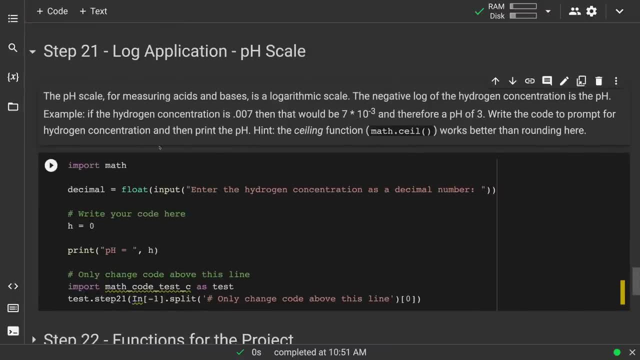 We get the idea. So that's really it, Just taking this, and if you knew the hydrogen concentration, I was thinking about adding this in as like going into the chemistry and finding hydrogen concentrations, But I'll leave that for those of you that want to pursue the chemistry angle on this. 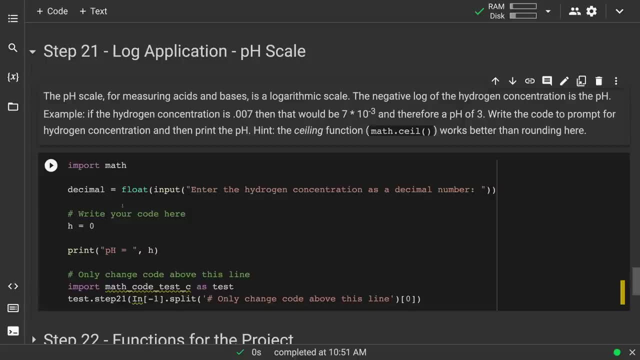 But you can. You could actually get various hydrogen concentrations of molecules and work it out from there. Okay, But nonetheless. so what we want to do is we just want the hydrogen concentration. So it's the negative log, And for this one, 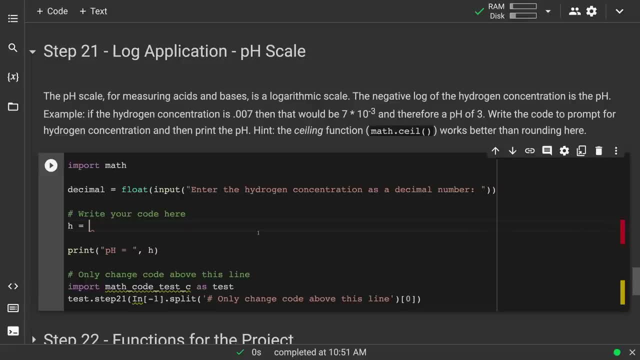 I will use math. So there we go. So we're going to make this negative math dot log And I'm going to log as decimal 10.. There we go, So that's really it. And now that log, I get that number base 10.. 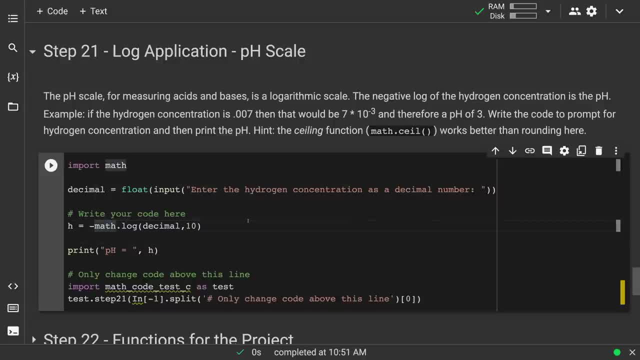 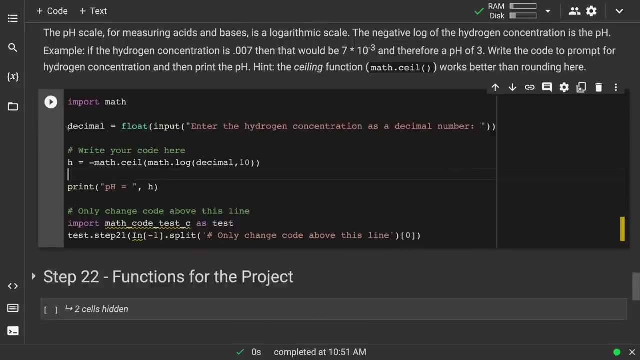 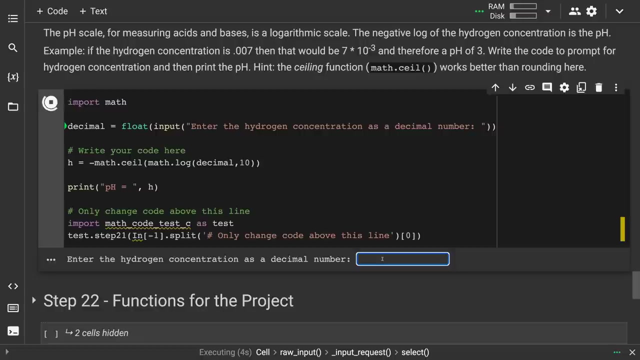 And what do I want to do? I want the ceiling, So I'll do math: dot ceiling of this. There we go, All right, So there we go. When we run this, I know the hydrogen concentration, And what if I put a point zero? 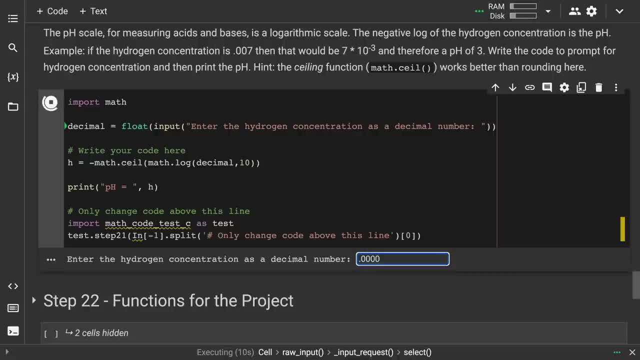 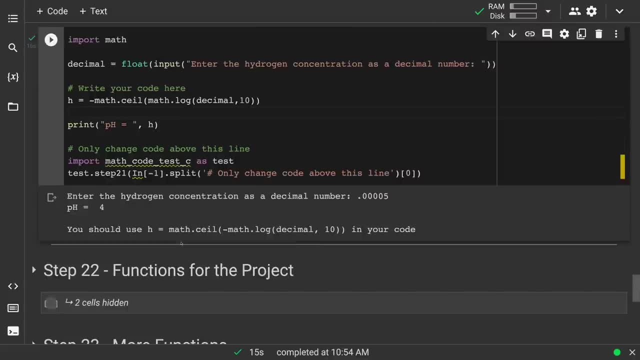 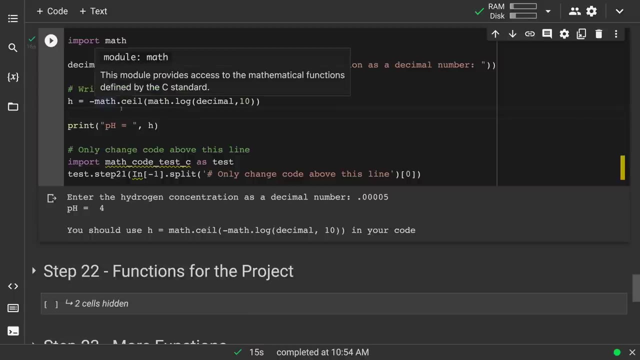 three, four and there we go And I'll put, let's put the number five. I could put a one there. Math dot ceiling: Yes, So I would take this as we. we look at this and, yeah, this is the function here. 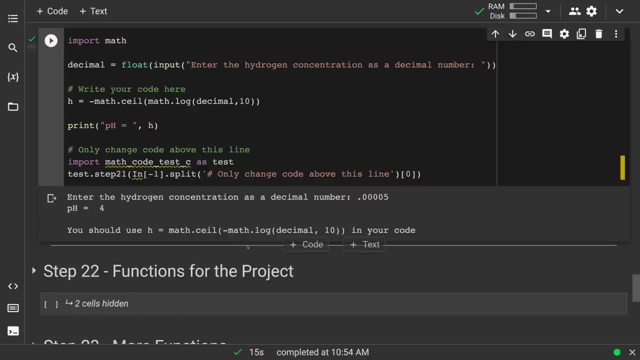 We run the function as is and then do the math: dot ceiling. So that's what we'll do. We'll move our decimal place And these are the things that I wanted to put in here. as you know, indications And you see. 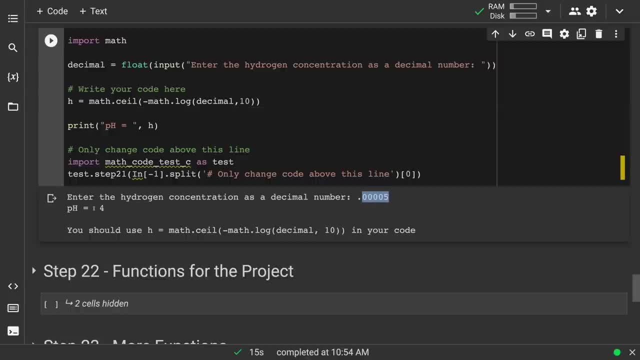 we see why this, this ended up being wrong, because then he gave a pH of four, putting the math dot ceiling In the wrong spot. All right, So I'll do the same same one here. point: I'll put a one. 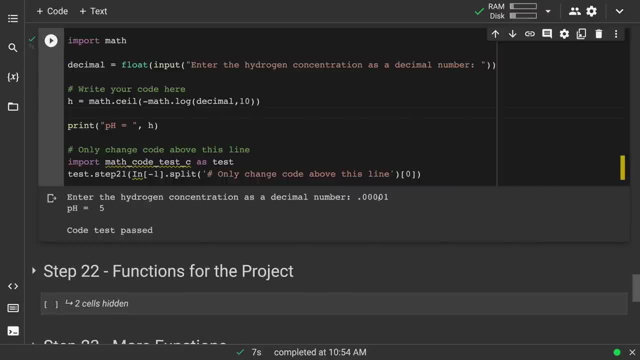 That's okay. There we go Now. that gives it a pH of five. You see how that makes a difference: Doing the formula first with the negative log, then doing the math dot ceiling. There we go Now. that gets a pH of five. 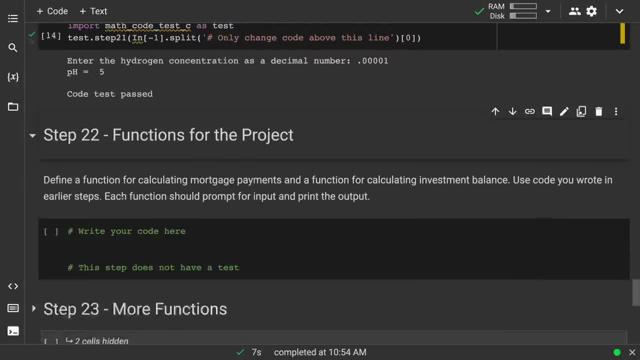 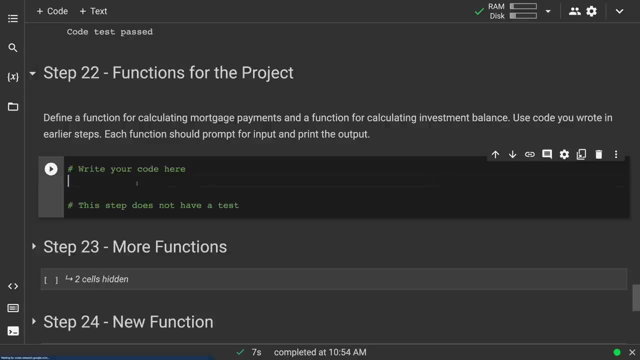 There we go, All right. So now with functions here. these are some of the things. How could we write a function? Well, if you want a function, you're going to define the function and calculating mortgage payments. Okay, So maybe I'll call it more pay. 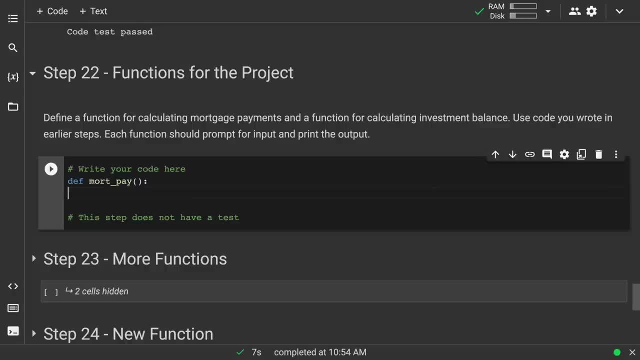 And now notice you would think that it, when I hit enter, it gave me the indent automatically. but for other things that I do or I might use this code. I am all about the four spaces, So I backspace, I delete that. 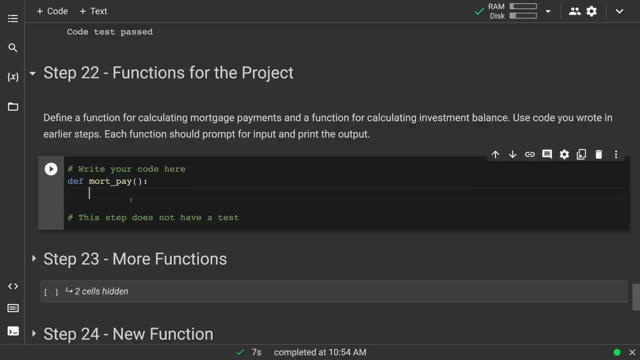 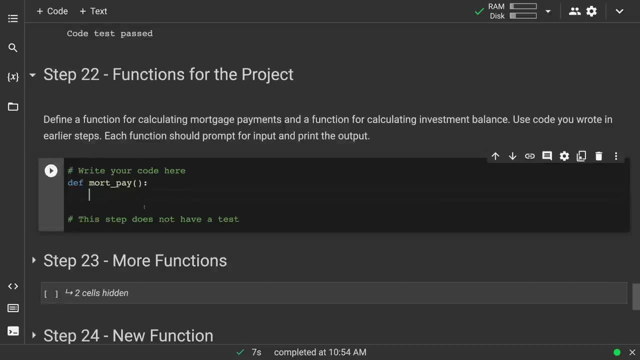 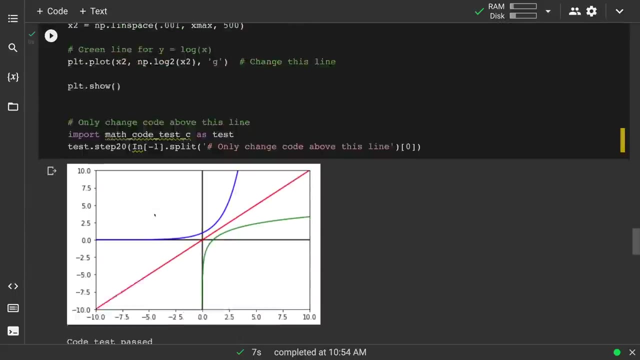 And then I want to make sure I do the four spaces. So what can I do? I can define this function here. So, and this is I'll do one, and then you can see how you can do more here. So, if I have the mortgage payment, 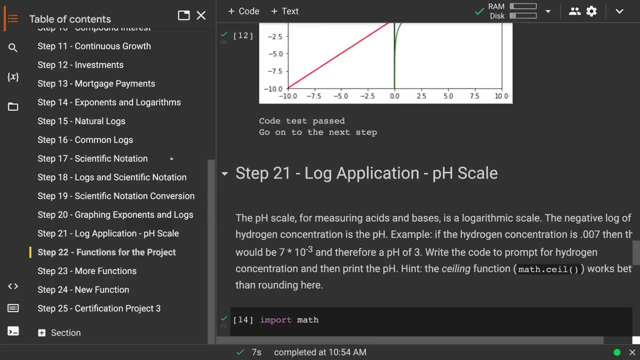 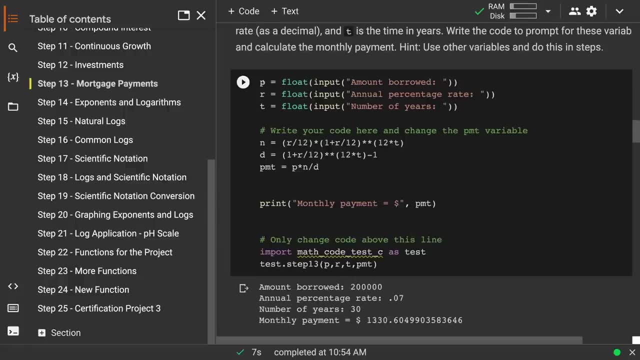 now we also have our table of contents. I can jump right to mortgage payments. So, notice, I have P, R and T here And then I will define these In here. So I'm going to just copy this and actually, there we go. 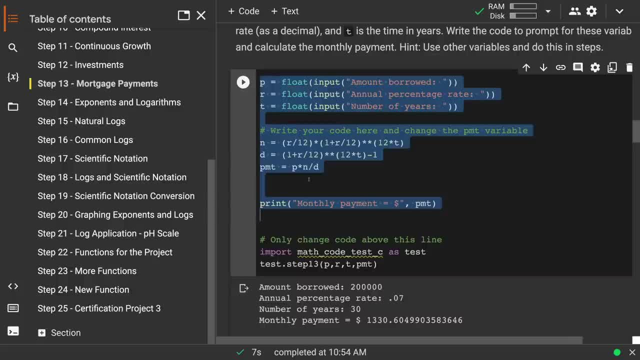 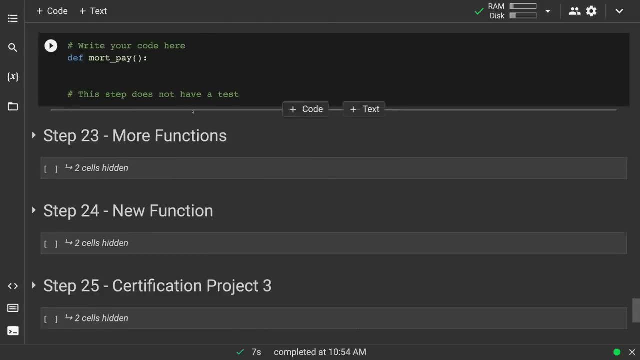 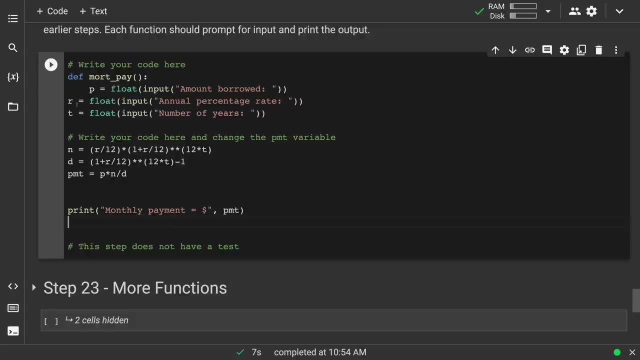 So I'm going to show you one way to do this, and then maybe we'll do it a different way. There we go, And more functions here. So one of the things that you can do is just put everything in here, And I might just 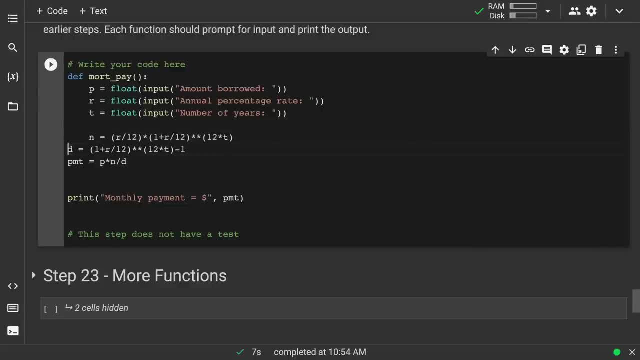 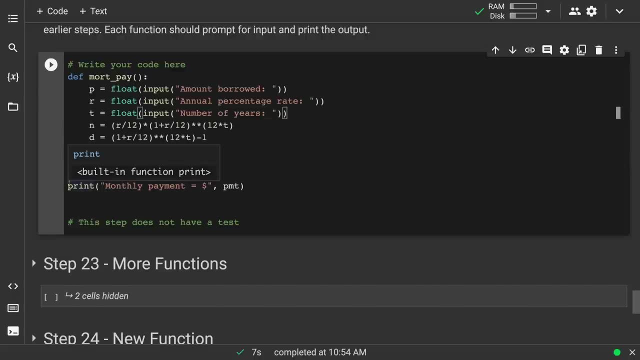 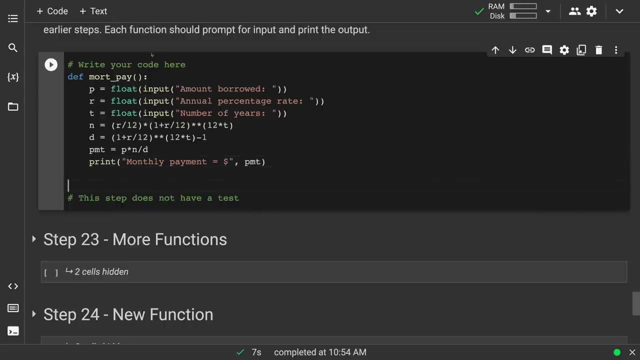 go. Probably don't need that extra line And same here, So this works As The payment. Maybe that's all you need. You want to be able to then prompt for these things and then print out the answer, So that works. 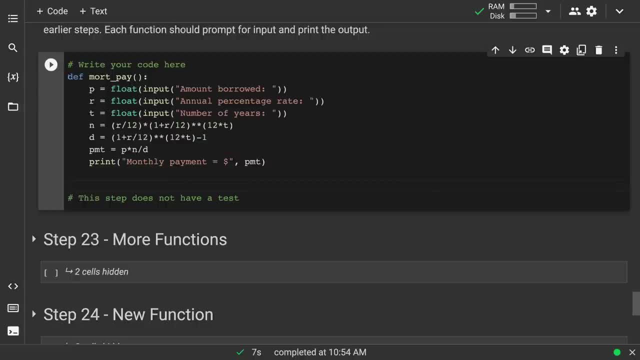 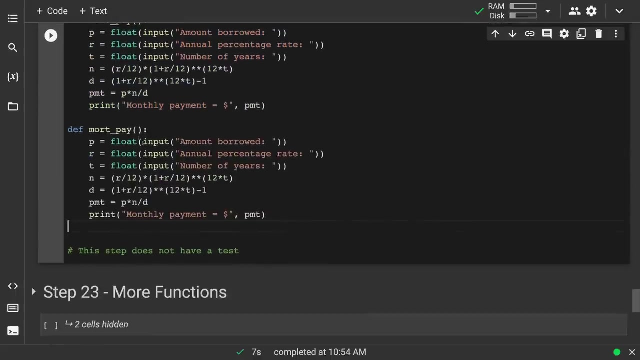 Another way Is What I'm going to do. I'm going to copy this And I'm going to show you another function that you can do And that one. All right, So more pay, P R T And for this one. 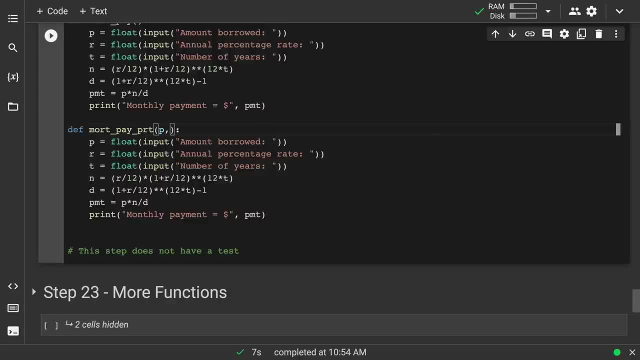 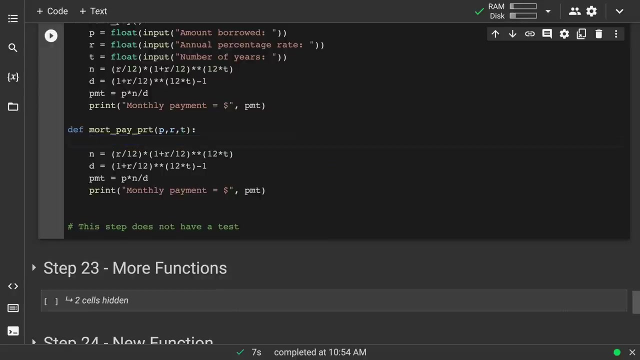 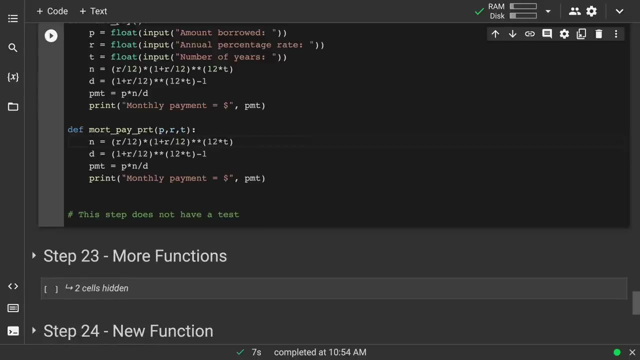 I'm going to require anything. You pit input P, R, T, And then I'm going to Not need these And instead of print I'm going to Return Payment. So This one's nice, If that's the if. 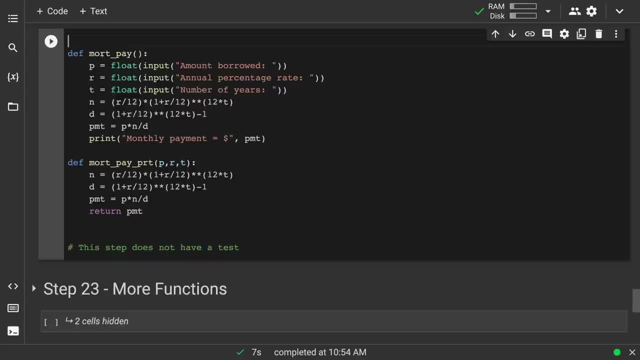 And You know, there we go, So this one's nice. If you wanted to Prompt, You know this could. This could go A lot of different places, But this one. You can put this in. Maybe then. 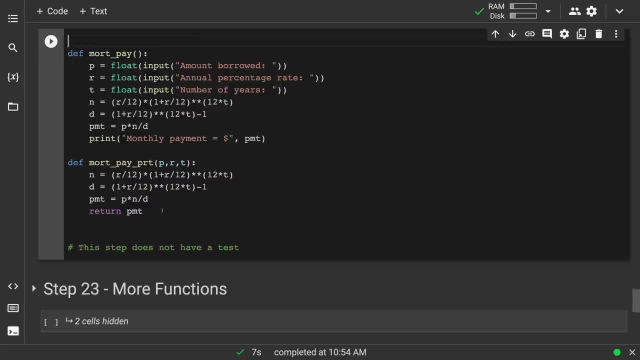 Just Put this function in And return the payment, Like exactly where You know It's going It's going to go. So Yeah, Two different situations, And that's why You know I'll make it, You know. 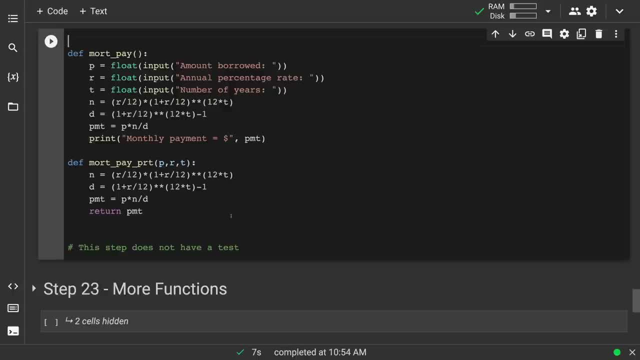 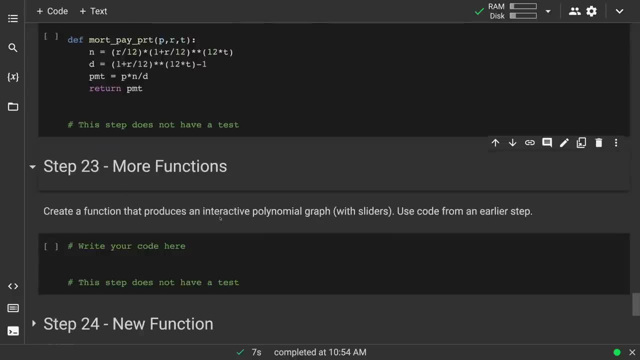 P? R T, So we know what the input would be, And then this one Is different. So there we go. So that's That's one, One way, And I have here More functions. Now I'm going to do. 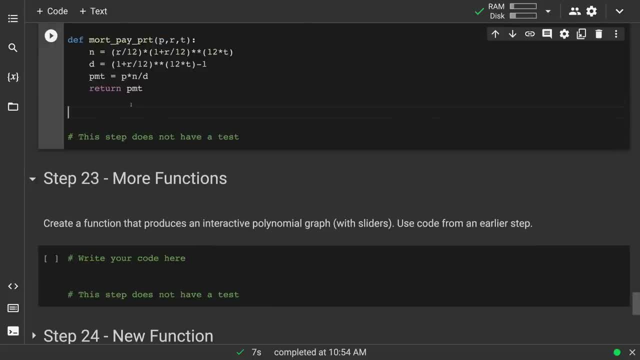 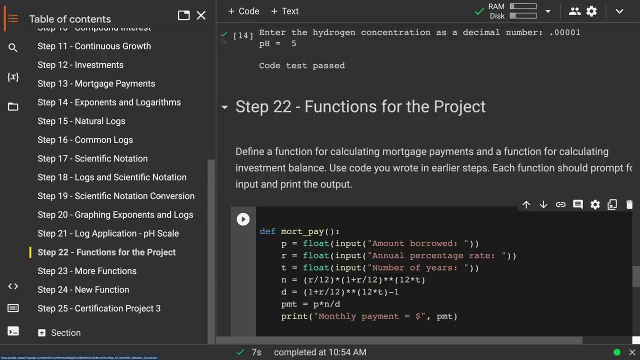 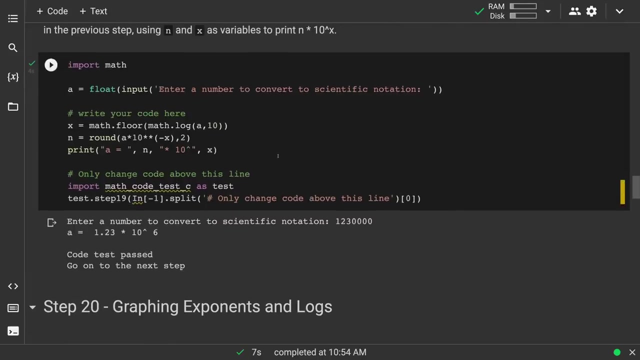 One more up here Because I wanted to Show you This Scientific notation. So Here we have Any Number to convert To scientific notation. So If we Have This, So If we Have, 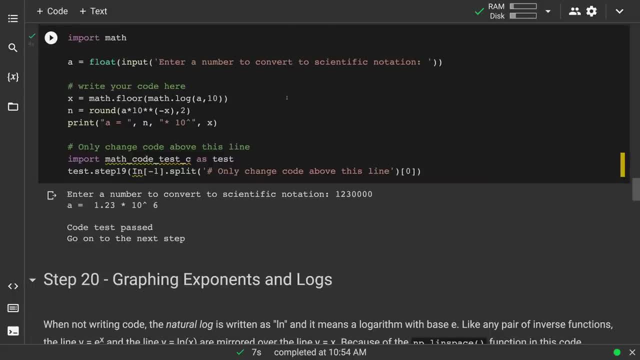 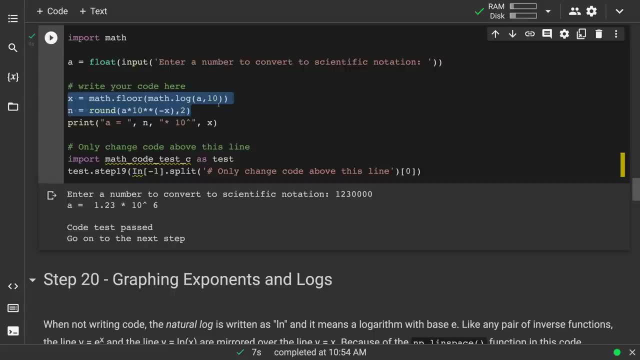 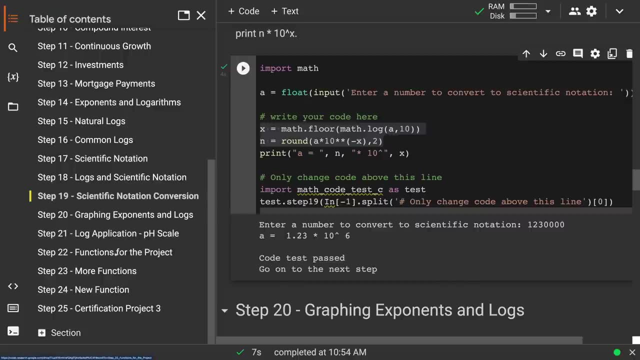 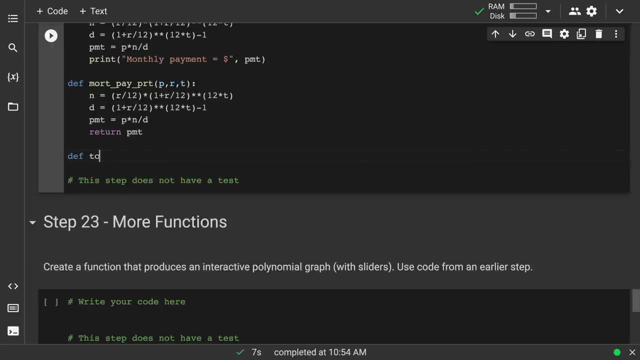 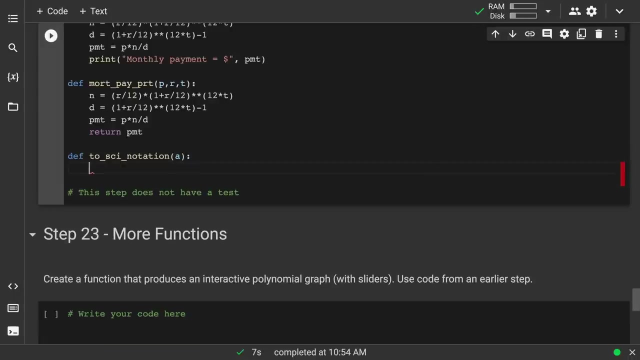 So There's my Scientific Notation. They're really Just two Lines And If I take That And Convert This I could, There we go, And maybe it just takes that input of A, There we go. 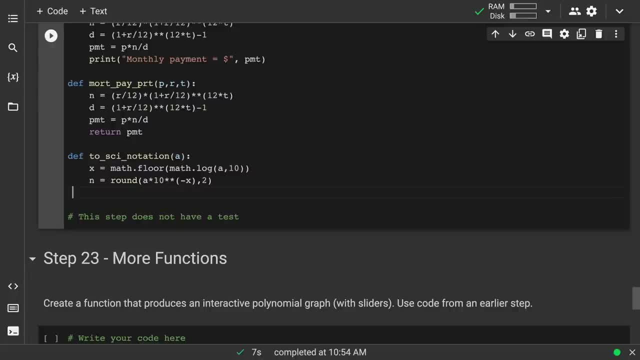 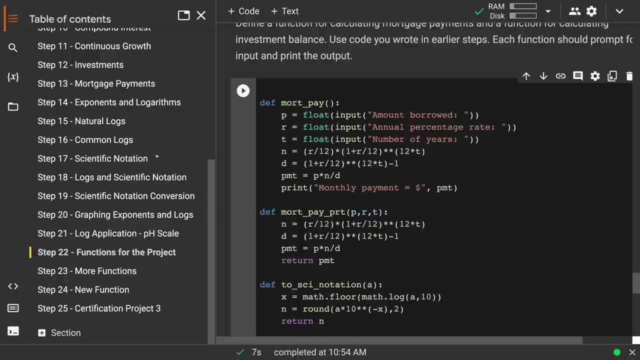 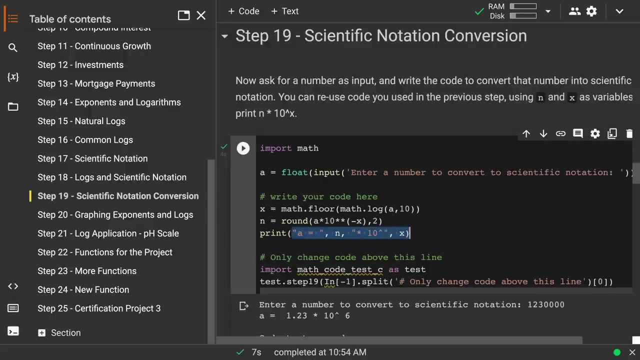 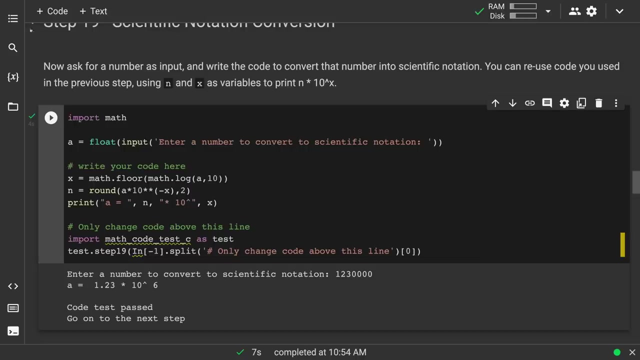 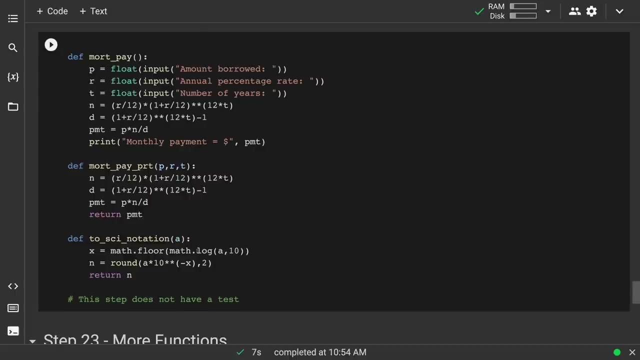 And return n. So that could work too. There we go, So we take this and we round. Oh, But I would probably have it as a string here, So I could go back to that And instead of the print, I could, instead of printing it I could, functions, I could. 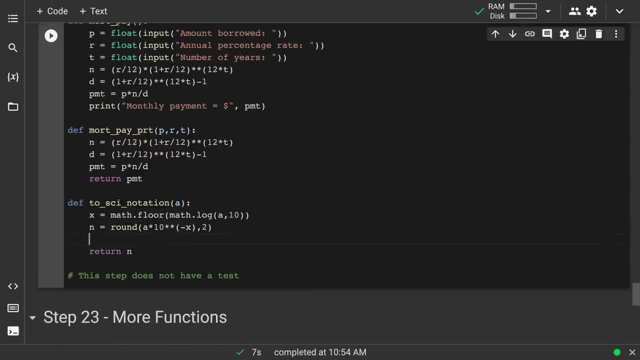 I could turn this into there. we go answer And so we make you know. I could just make that a string and then return answer. Okay, So I probably don't need this. A equals and it should give you n times 10 to the x. 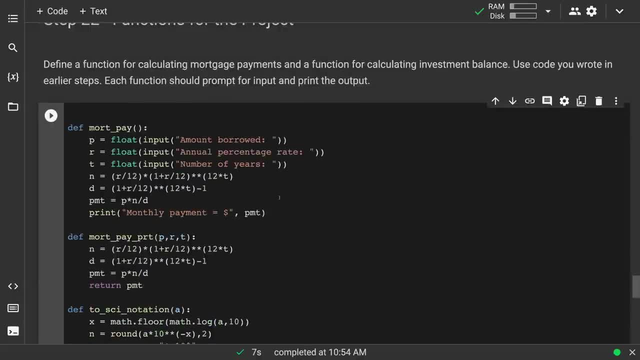 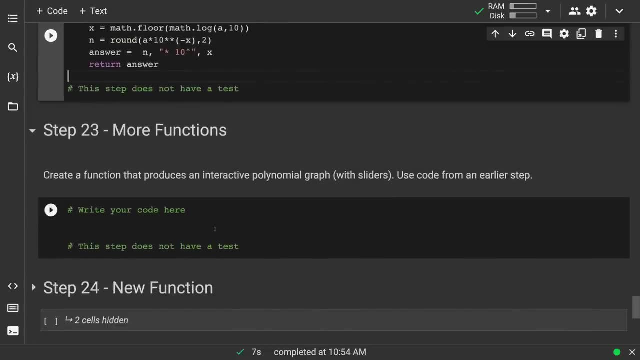 So, just to give you some examples, this is where I want you to be able to You create the functions, And then the interactive graph with sliders. We have that, So turn that into a new, turn that into a function. But here here's the examples, how, how you can just take, and that's the whole thing. 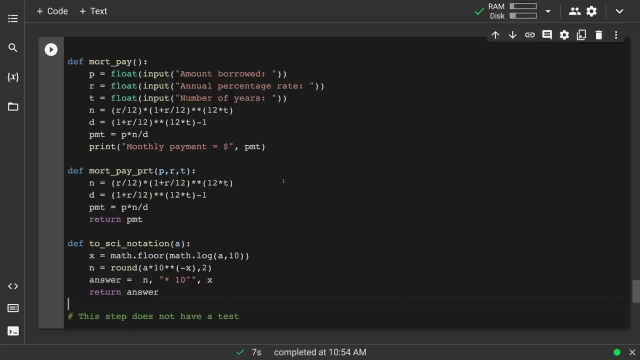 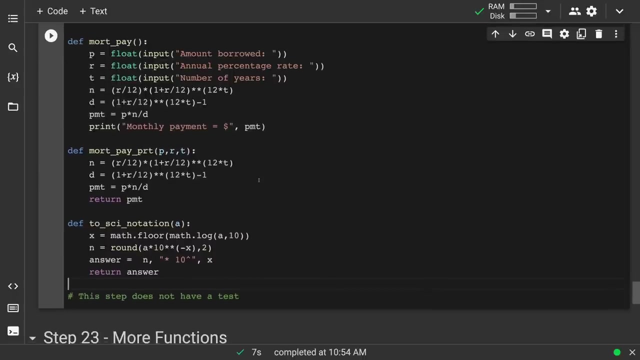 that we wanted to get to you know. through this course you're learning, you're practicing and then you're grabbing the parts that now you know and you can turn just the important parts that you're going to use later on into their own functions. 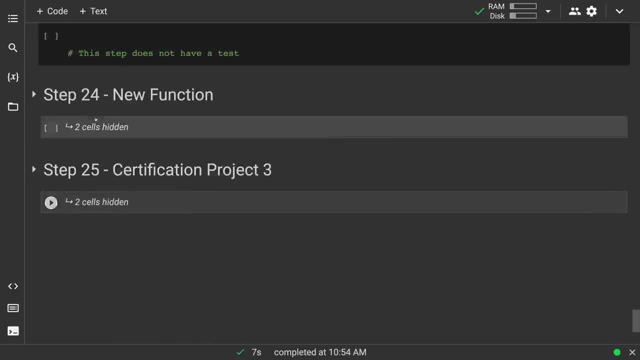 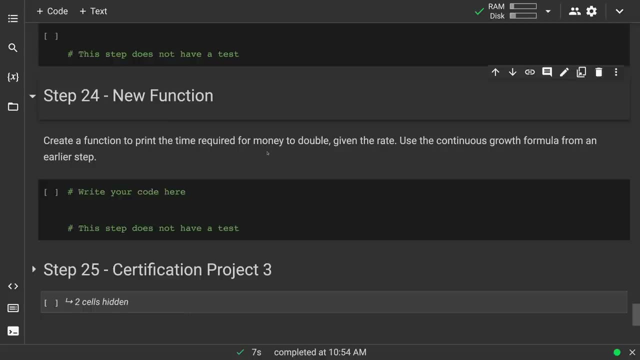 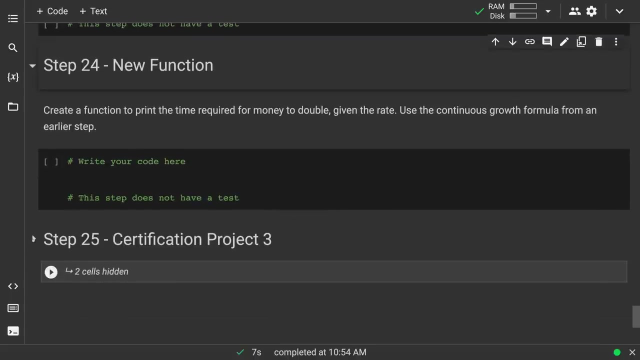 And you can, you know, give them other names. you know here's more functions and there we go. Create a function, for you know how long it would take money to double, go back to that other one Again, turn that into a function, and all of this is going to be in a financial app that. 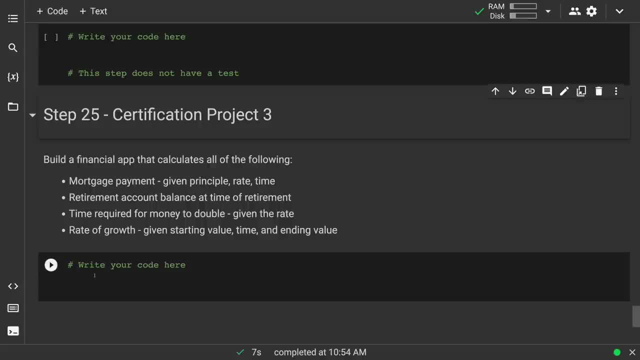 you'll make. So what you can do is you can have um one display of all of these and you could have this workout that it's within all the code here, or you could have it within, uh, within Google CoLab, where you have text that gives you like number one, calculate mortgage payment. 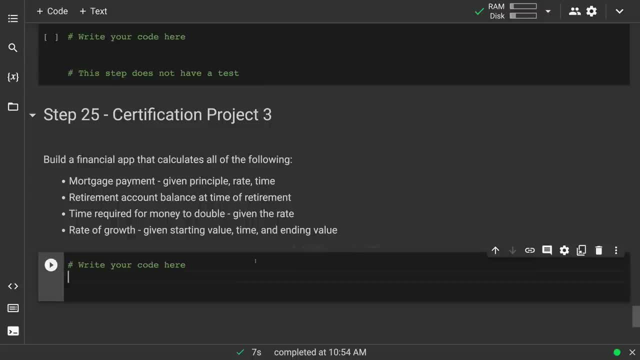 Number two, retirement account balance, Number three, et cetera. You could have the text there and then require input: which option do you want? and then have all your functions. So that's that's one way to do it: Defining all the functions, having the text input. that would be like the menu. 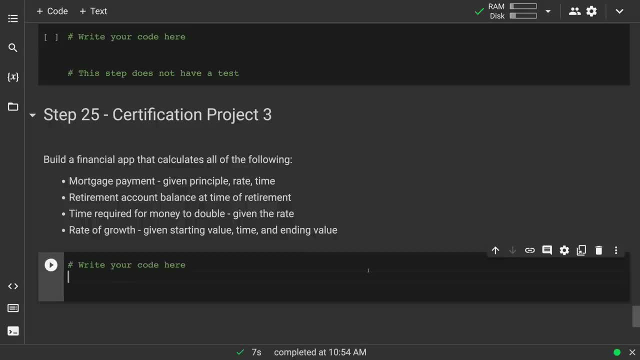 And then when you pick your option, then it runs that function. So that that's really what I want to get to, is that you're putting all this together And it becomes your financial app so that you can use this for other things- calculating. 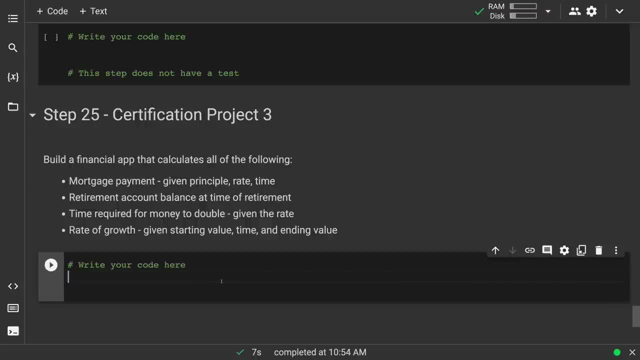 your own finances, And this combined with what you're doing in certifications one and two. see now where the goal is: that you're getting to the end of this and you have understand the math and you have all these functions at your disposal, You know. 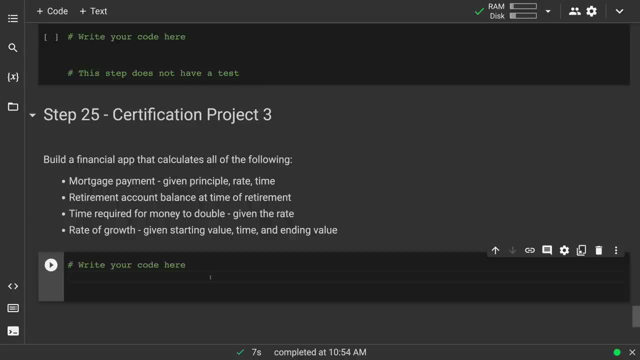 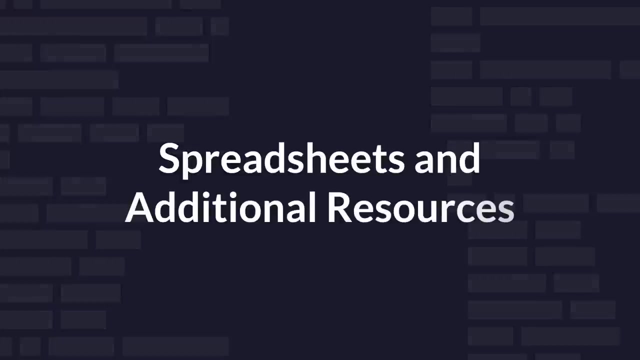 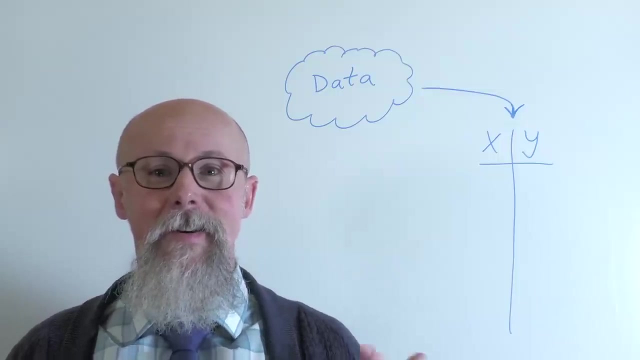 Calculate things, graph things, solve problems, and then you can apply that later. So the next unit, which I called week 15, is going to be the wrapping up and putting all this together. So we reached the home stretch in our algebra journey here and now we're going to connect. 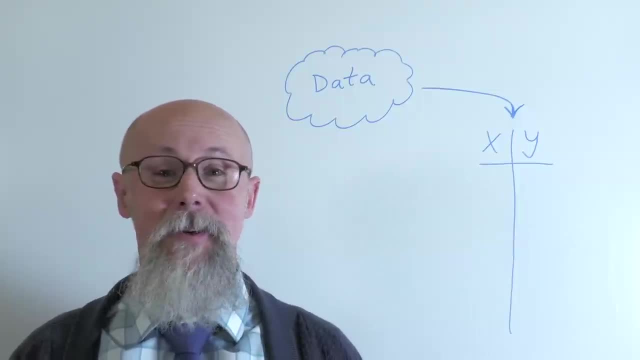 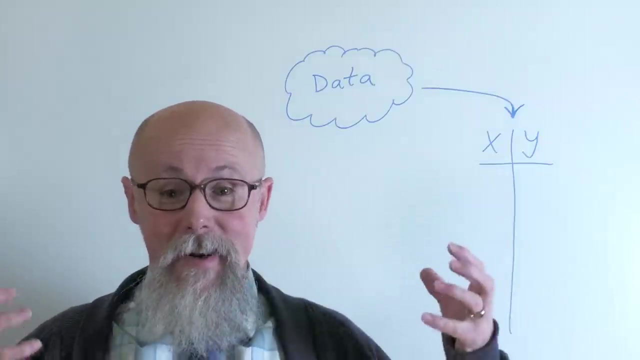 all the different things we've been doing with math. We've been looking a lot: Okay, Okay, Okay, Okay, Okay, Okay, Okay, Exactly Perfect. The last accumulator was bit favourite one, Correct, Correct. It's like: Oh yeah, that's the last episode of frustrating math. 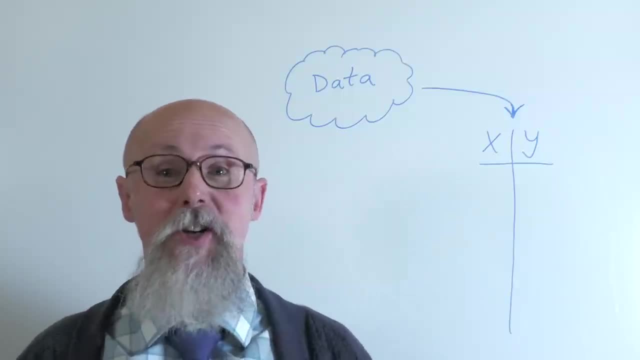 So time to treat this a little easier. This is actually my second time doing this. I'm learning kind of new 2d math. then we can do math to it. So really that's the connection We've been working with all the math. 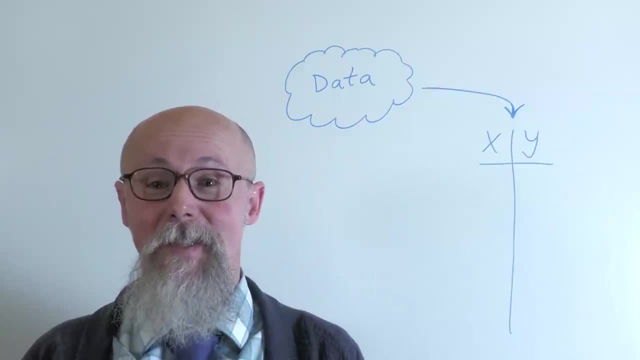 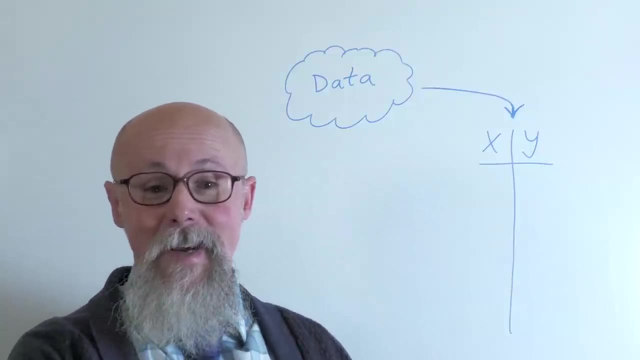 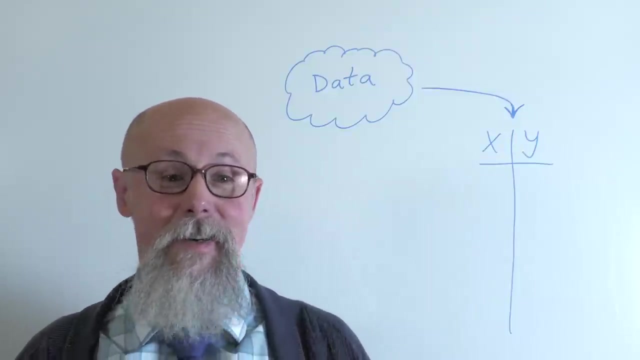 content and now pretty much everything we're going to be doing beyond this. we're going to bring that math content into the code and do a lot more code. How can I get this data, turn it into a NumPy array and then do whatever graph I can do and analyze the data. So let's get to it. Let's get. 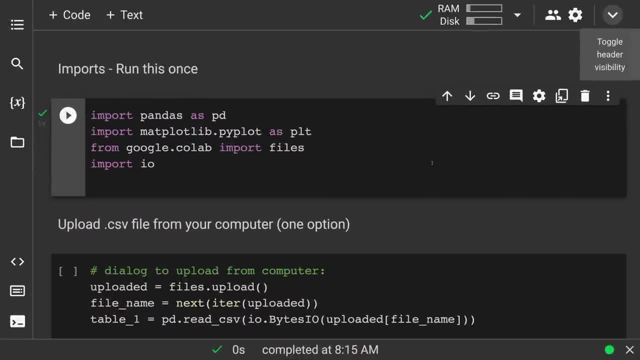 to the code. So now, this is some ways you can bring in data from other sources and graph it and do other things. So let's talk about the other sources. Pandas is the library that really deals with data- frames, tables, columns, rows, everything like that. So we're going to import pandas. 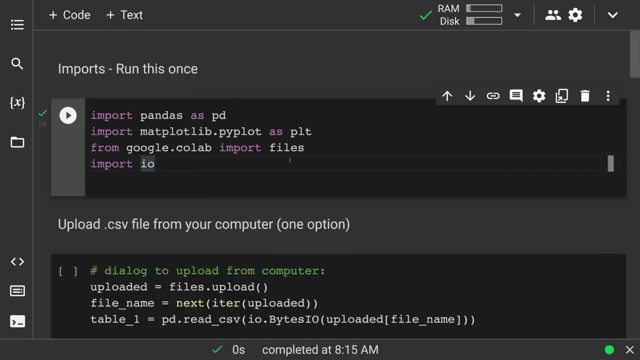 import the matplotlib. we've done that before and we're also going to import the matplotlib. We're going to import from Google Code Lab. we're going to import files- That's also going to give our file operations, you'll see that- and import i-o input output. There we go. I separate these out. 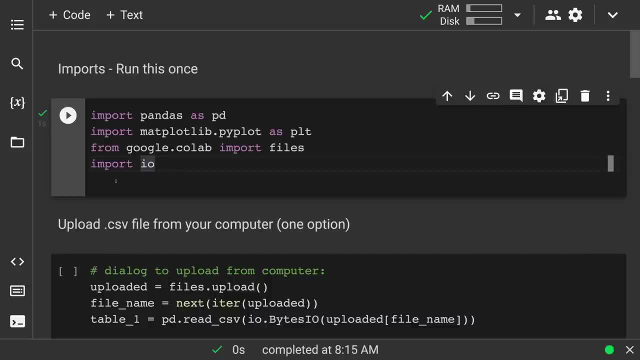 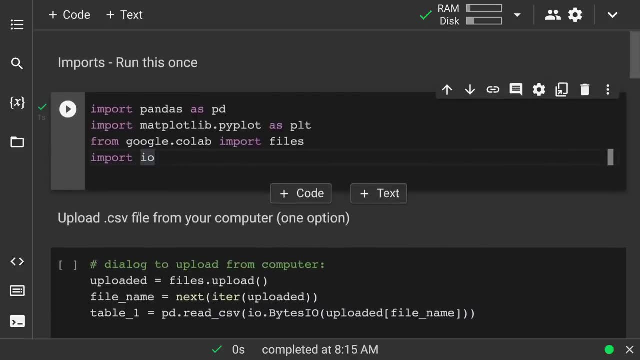 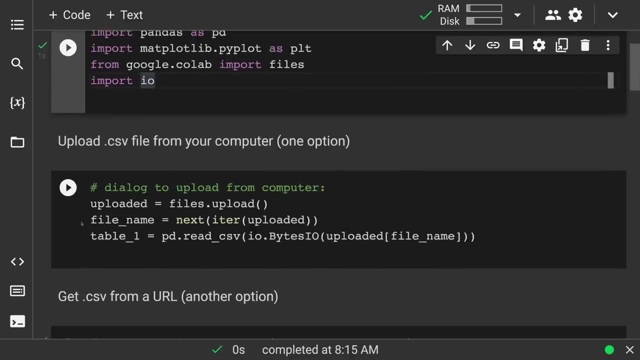 because you can run these once and this takes a few seconds. I already did it, So run it once and that saves you a few seconds each time, because we want to go through- you'll see- test some things. Now we have all those imports. here's ways that we can get the files all right. here's one option. 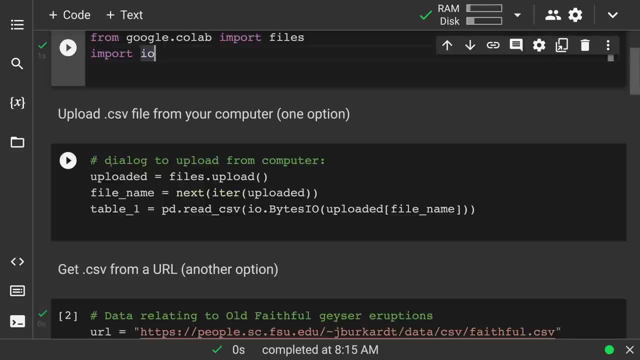 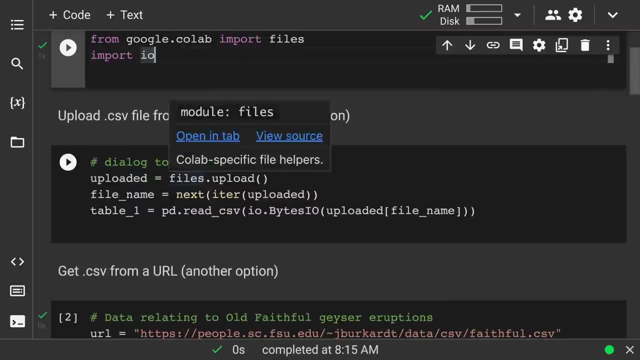 if you have a csv on your computer, you can upload it and because we imported that google dialogue or the google files, all right, so this is all we need um filesupload and we're going to upload that. you know it'll give you that file dialogue. you can search for it on your computer and 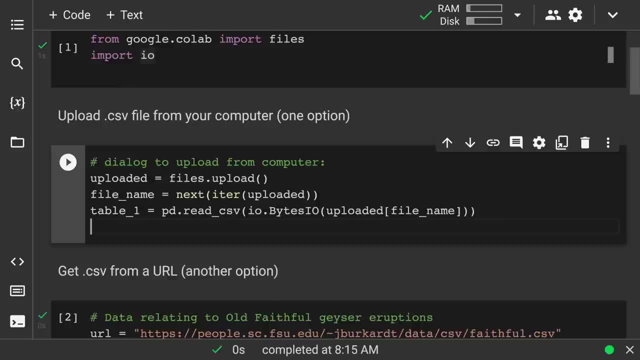 that's what the one you select will will store that as that variable uploaded and then so i have my file name because we have this. we're going to take that uploaded file and iteration, so iter and the argument is uploaded and we're going to go to the next one and what that is going to do. 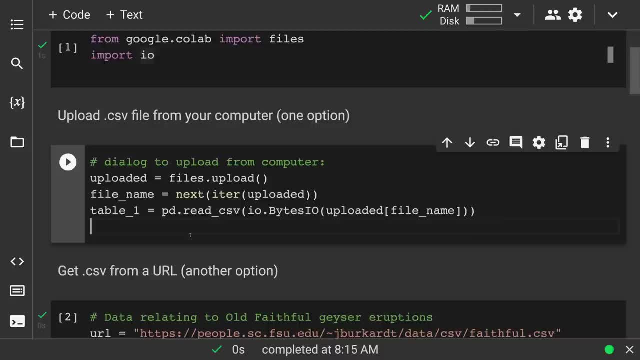 is just one time. you know you selected a file and we're going to select that and store it as file name. you and here that file name. we know the file name and we know that it's a csv. so pandas has this nice building pdreadcsv. that's what we want to get to and don't worry about this, it's because 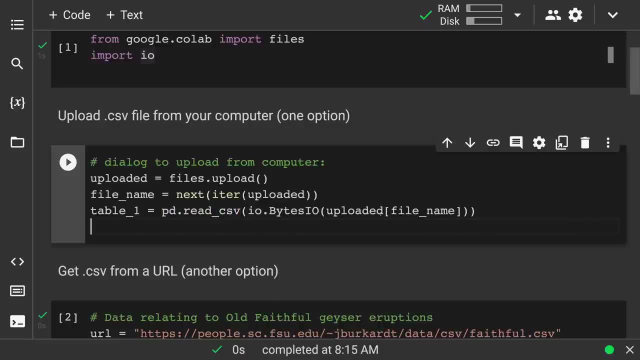 i already stored that as file name. you can use this for you know, whatever file you upload. so uploaded file name and it reads that iobytesio, and it will store it as this table. so there we go, these three lines from you know, uploading something you know. give you the file dialogue, upload it from your computer and select it. 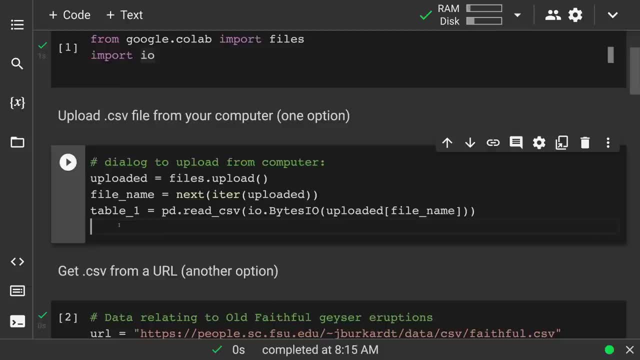 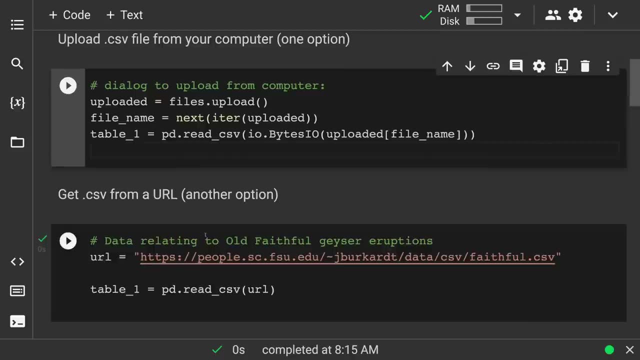 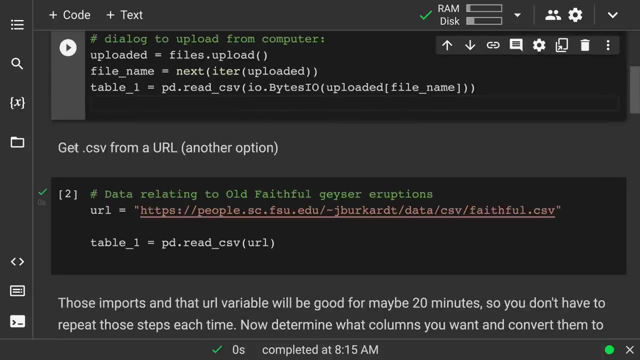 now, when you run this, when you select that file, it's stored as table one. awesome, so we'll. we'll do more stuff with that table in in a minute here. another way is you can get a csv from a url. so maybe you already know you're. 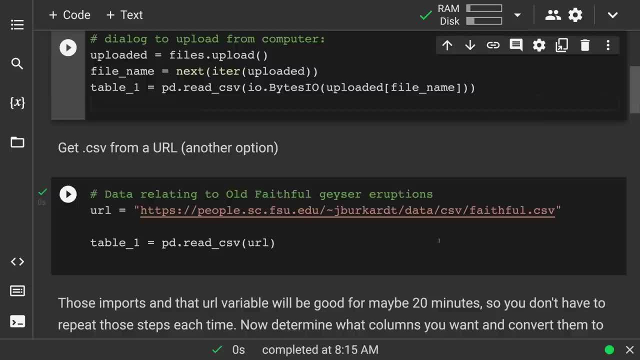 looking at different websites and you found you know this uh url and you see um this one, um, uh, yeah, this, this guy uh seems to put put out a few good examples. um, so there we go. uh, faithfulcsv, old faithful geyser, um, you know, erupts from a little, you know briefly, but like on such a regular. 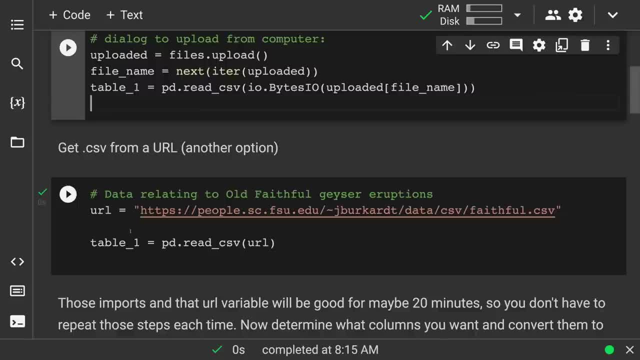 basis. that's why it's called old faithful- and that just might be some interesting data we can look at, so i'll just store it as this variable url, which is the exact address pointing right to the csv. there you go. plenty. you could also- and i didn't include this here, but you could also. 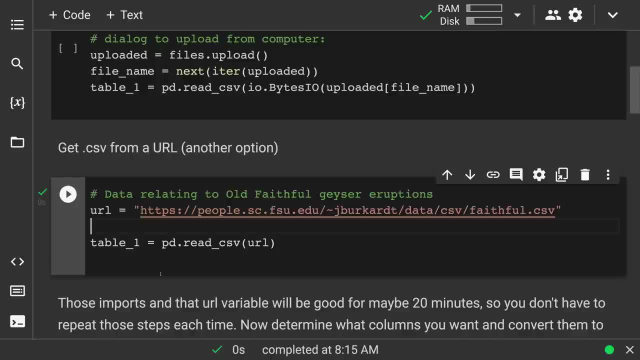 if you wanted to, you know make your own, like you know. input statement. you know prompt, you know for somebody else using. you know you made this program for somebody else. you could prompt somebody else to just copy and paste the url and store it. you know that works too, but you know this is your code, so you just put the url here, store it as variable url. 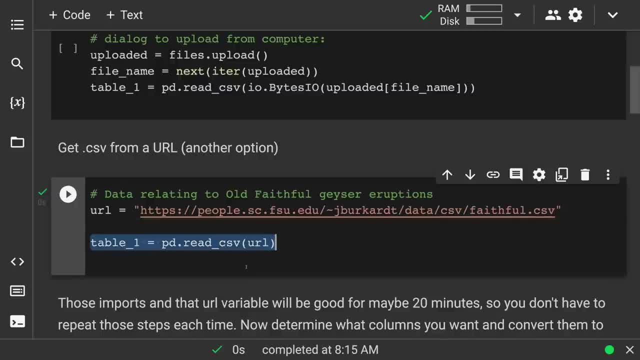 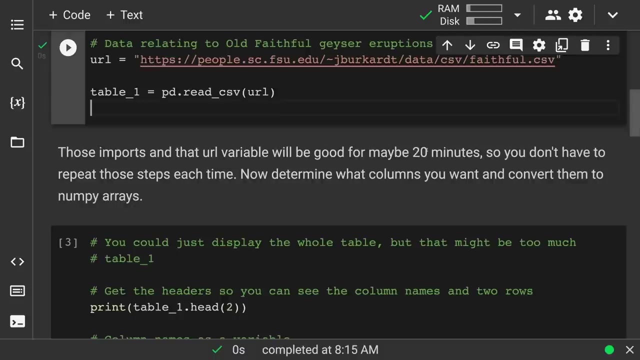 now same type of thing but here. so we have pd- uh, because we imported pandas as pd, pdreadcsv, and i just need to read that url and that's enough and i'll store it as table one. okay, and yes, those imports and everything that you run, um, i just even have notes in here to 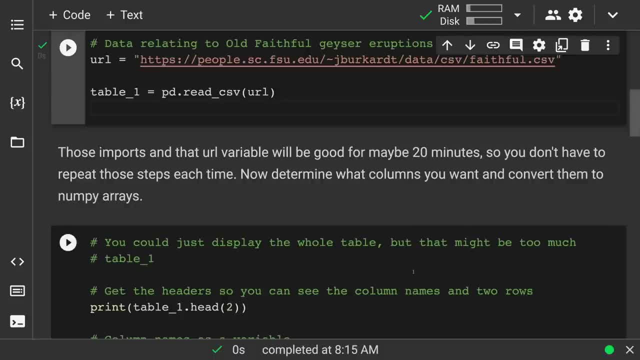 remind you. so that's good for maybe 20 minutes. google colab will, uh, have this runtime. you're running on their server and you know colaboratory has a runtime. once we started this, it will time out after about 30 minutes of inactivity, or um, even if you're active, like you know. let's say: 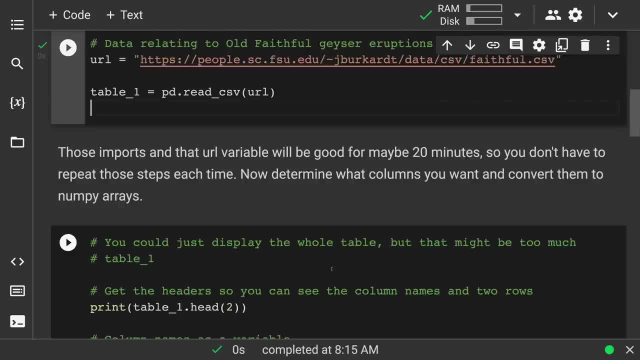 you have a really busy day. i think it's like about 12 hours of running, it'll time out. you know you could say, well, wait, i haven't been inactive, but there's still an absolute time out, and then you have to start it again. so that gives, that gives you time, you can import that, and then it gives. 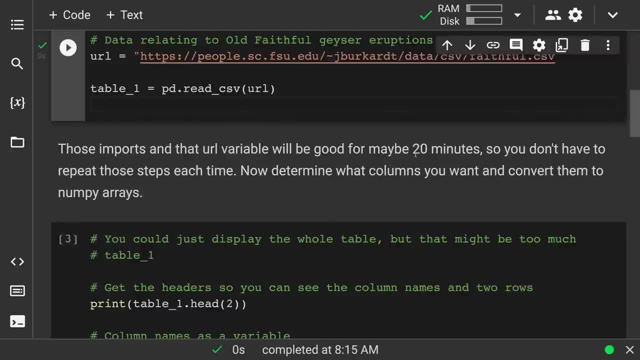 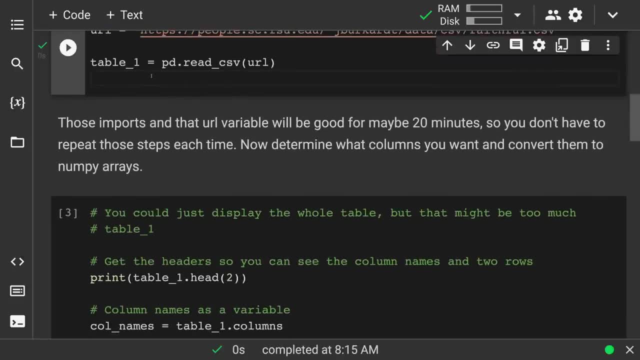 you time to go through and import it, and you can import that and then import it, and you can import the and run a few of these and tinker with it. Okay, so that way you don't have to repeat those steps And again importing all those. 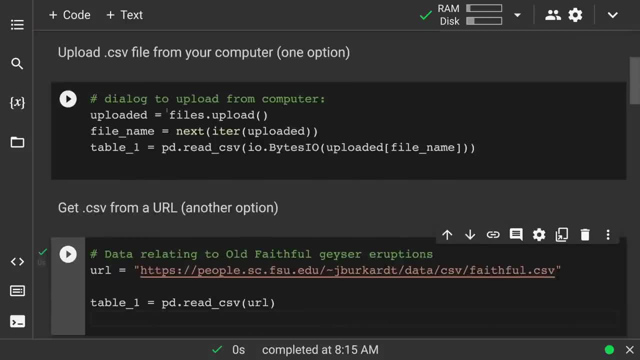 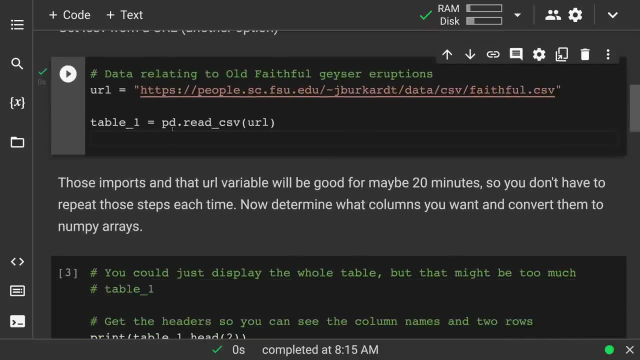 that actually takes a few seconds to run it, And then prompting if we want to do some different things and test some things. you don't have to upload it every time. That saves you a few seconds, or this. even So, there we go. 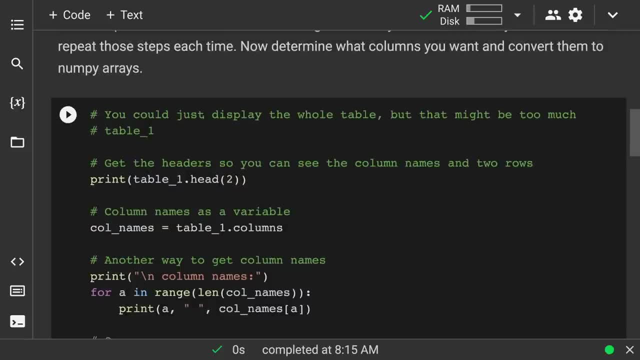 Now we have this. What do we want to do with it? I have it in the notes. We're going to eventually determine what columns we want and convert them to numpy arrays. And remember, numpy arrays. that's what we end up graphing. 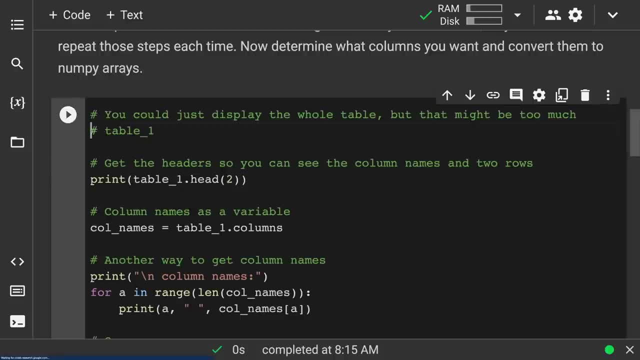 So one of the things- and I even still commented this out, but you could display the whole table- That might be too much, Especially the more you get into big data. that's going to be just time Consuming, resource consuming. 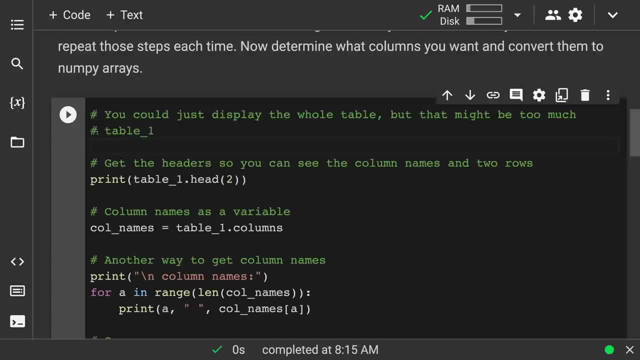 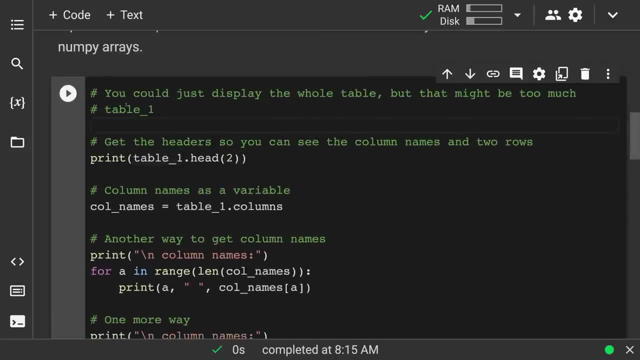 And so I include that in there just to show you can do it. But what else might we want to do? I might just want to print out. So we've always stored everything as table one, for this example, So I might just want to print out the headers. 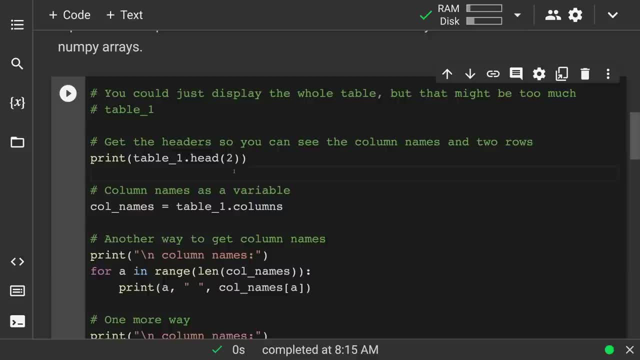 All right, so table one dot head And if I don't put a number in parentheses it will default to five. But I can put a number in parentheses. But I can put a number in parentheses. But I can put a number in there. 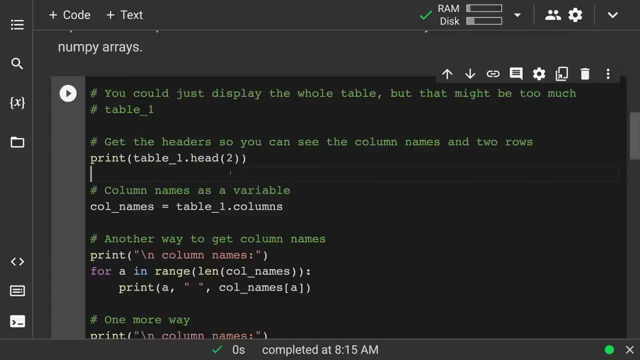 And it's going to give me the headings and I put a two, So it's going to give me the headings in two rows. That might be enough. Let's say, even if you've seen the column, you might want to see it here. 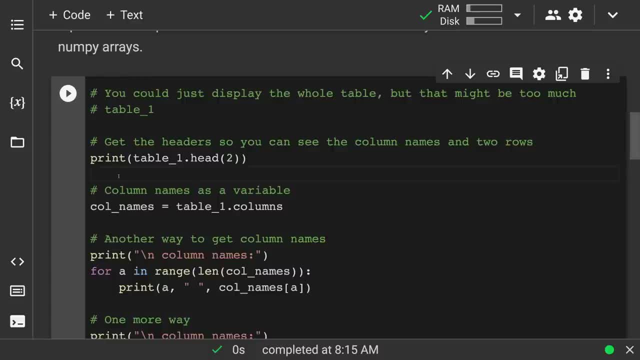 Or you got that URL. you want to take a look at it. I want to see the heading, I want to see the column names And I want to see two rows. Give me an idea of what kind of data, Because if I start seeing words in there, 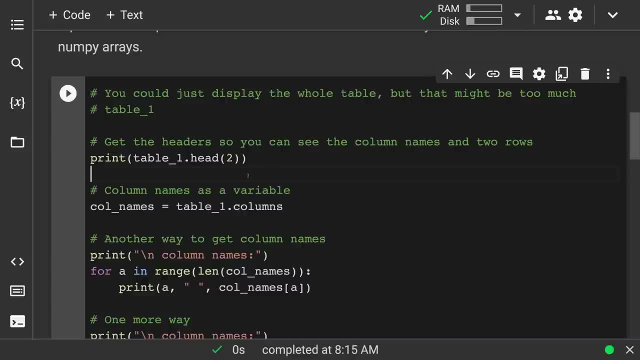 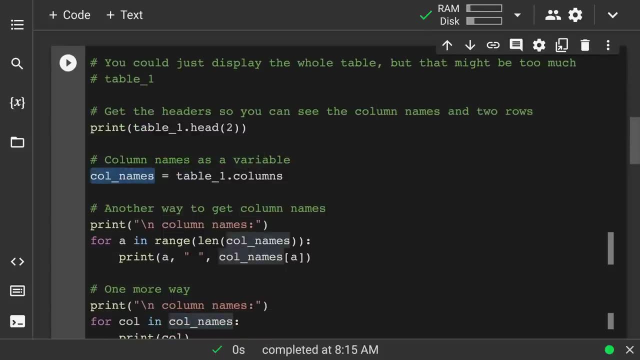 then I know that I'm not going to be able to convert that to a NumPy array. All right, another way: I could just store column names as a variable, Because if I have table one in pandas, this exists: table one dot columns. 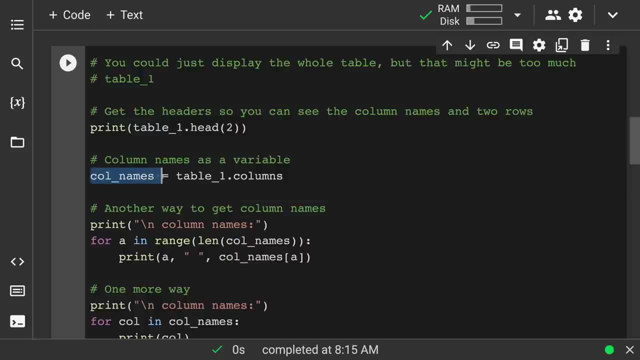 There you go. So now this column names is a list of the column names. That's great, And again, I only need to do this once. And now that I have a list of the column names, what can I do with them? 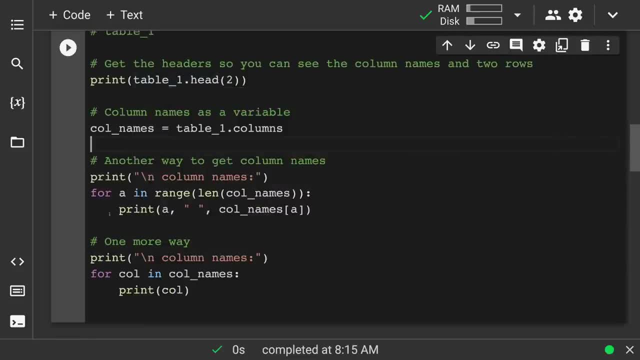 All right, Instead of printing out the heading, I could and I just put this here. you know new line column names and then I could loop through them, So I'll count them. So a in range length column names. 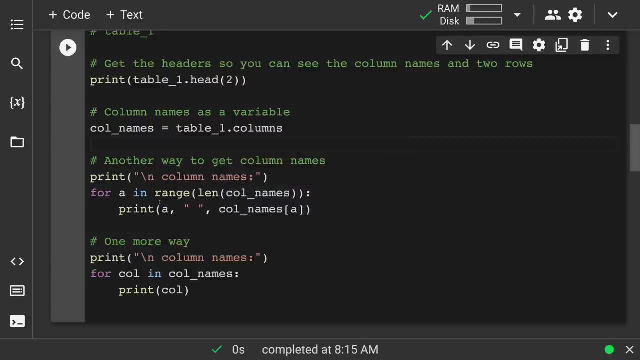 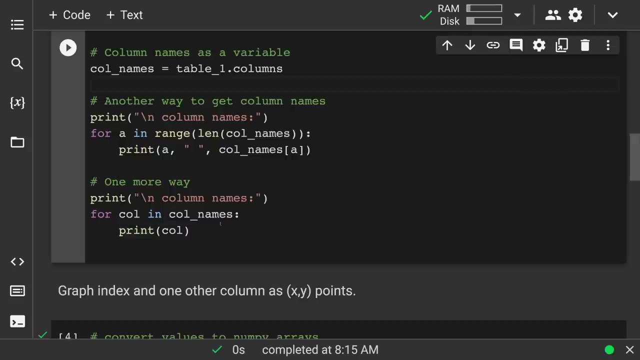 So column names. I'm going to get the length, Get that as range, And then each time I'll print that number, The space and then that column name. that works. That's one way to do it, Or another way I could actually just loop through those names. 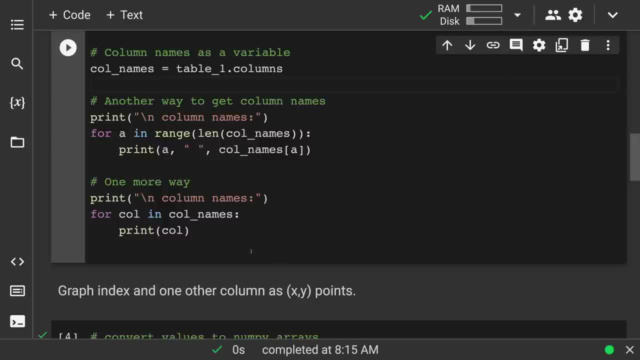 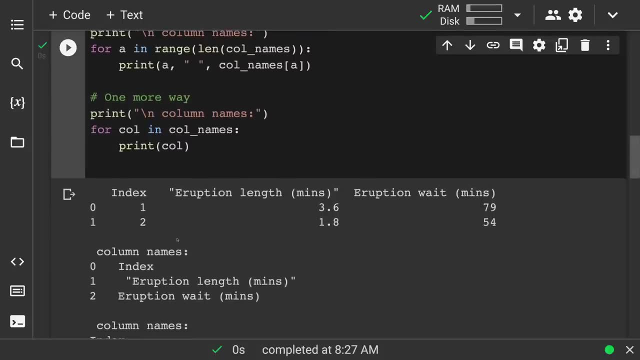 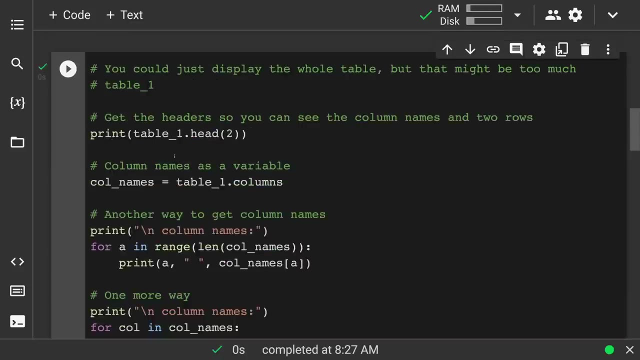 column, column names and just print that each time. So let's see what that looks like. All right, And so these are the benefits here. So notice, this is the first one we did. There we go. Print table header. 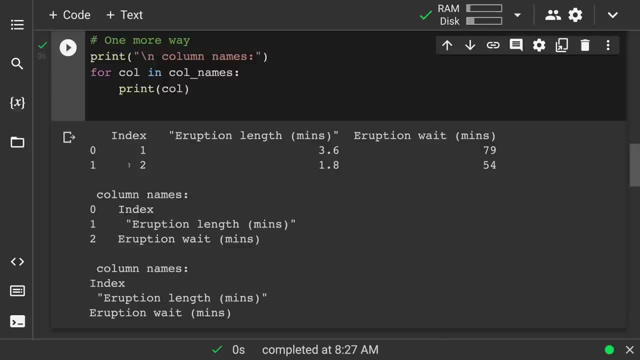 And that print statement, that head statement, gave me these. but this table also had an index column And notice their index starts at one, So that's just something to remember. And eruption length and eruption wait time. So there we go And notice these quotes are: 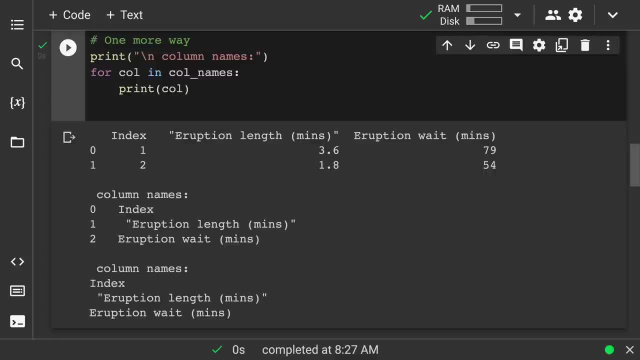 are within the within the name of the column. You know that's something. the more you get into working with data and maybe other people you know creating columns and everything, I'll tell you this: you really want column names without extra. 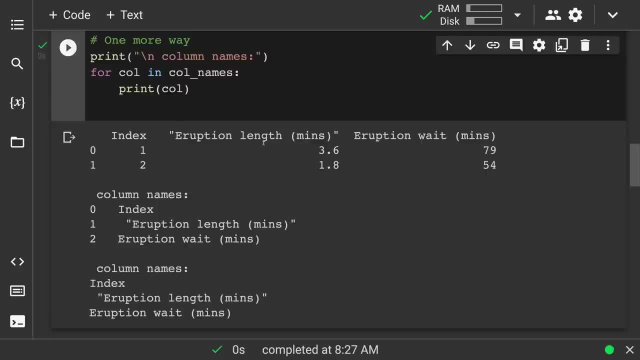 quotes in them and without spaces. But you know there's ways to deal with that, We can do this, but it just, it just usually makes it easier for this stuff And for, like, some of the SQL queries. Okay, So now I get an idea of what I have. 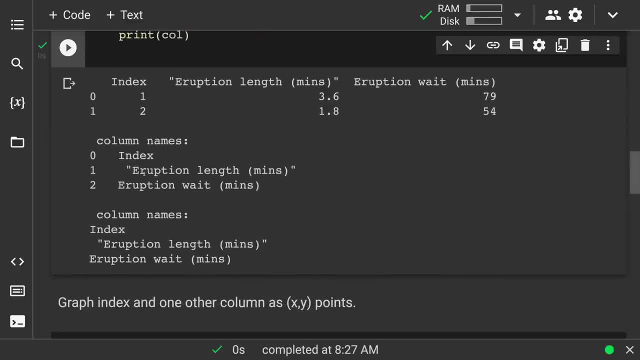 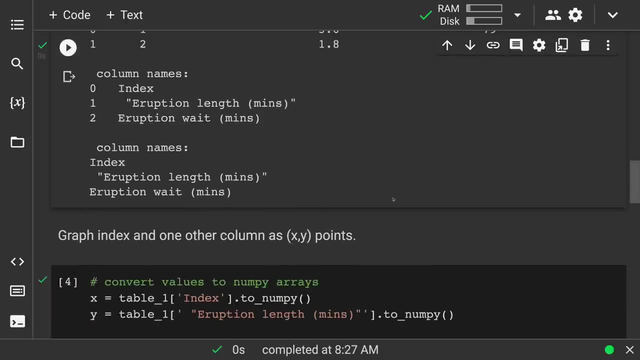 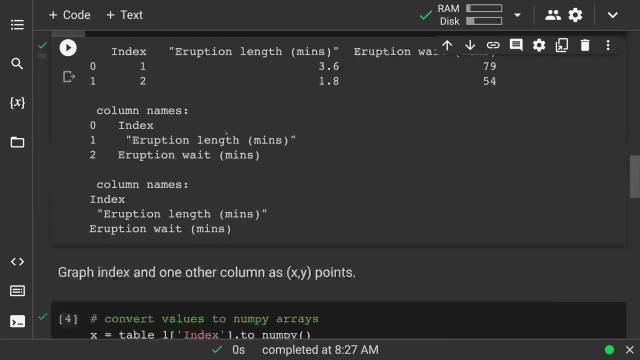 And here again you see the column names. you know index eruption And the other way we did it: Index eruption like eruption wait time. So now that I have these exact column names, So You know I could- now this is how I did it here, because I had them right here. 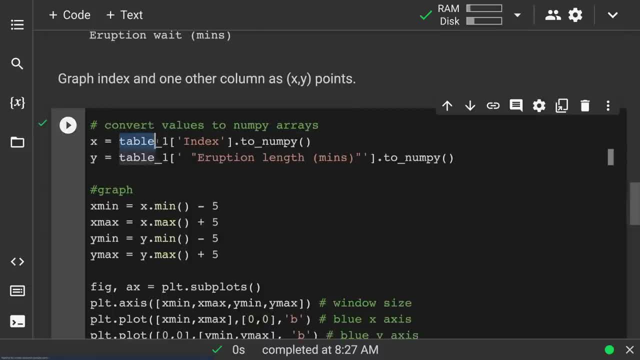 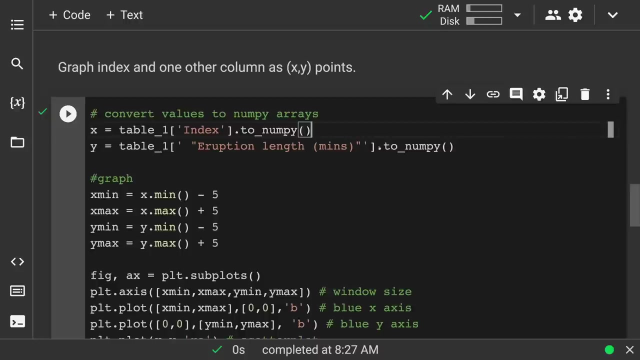 And I can. Yeah, see them. so table one, and then in those square brackets i'm going to put the name of that column i want and then also that name in single quotes to numpy. so boom, that'll convert that to a numpy array and then eruption length in minutes. so again, table one, and then in the square brackets. 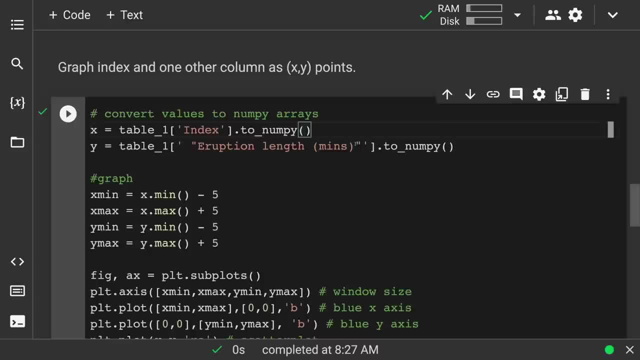 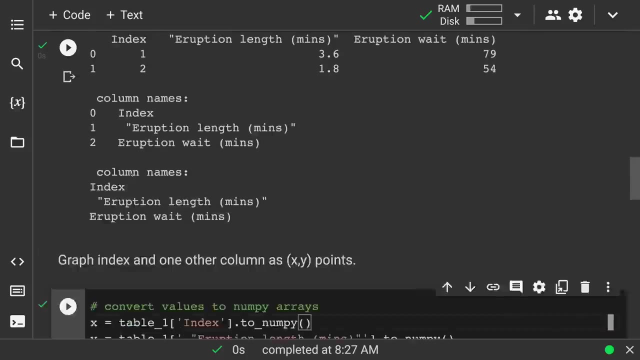 and remember that extra space and those quotes were in there, so i need to make sure i include them and convert that to a numpy array. so now i have my x and y values that i can, that i can plot there, you know, going through each of them, you know it's going to be, you know, my first value. 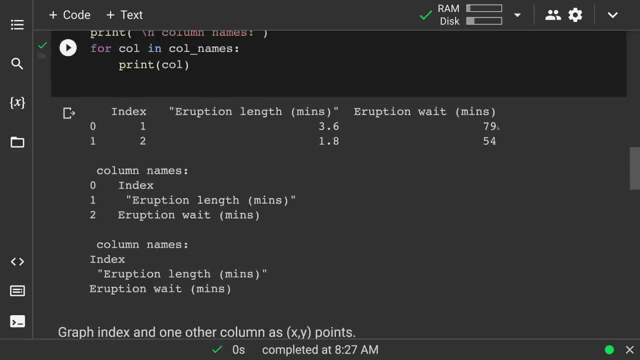 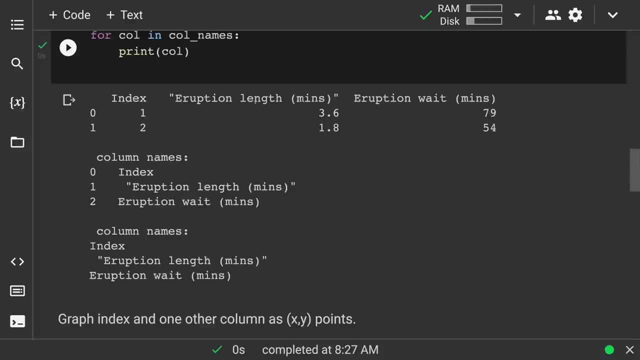 x is 3.6, y is 779 um. x is 1.8, y is 54 um um um. actually i had it as index, so x is 1, y is 3.6, x is 2, y is 1.8. i can graph the eruption length. 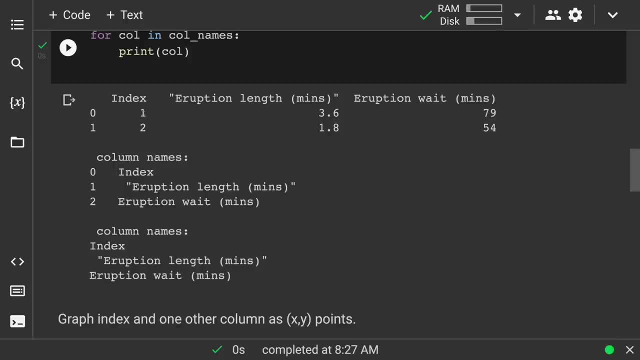 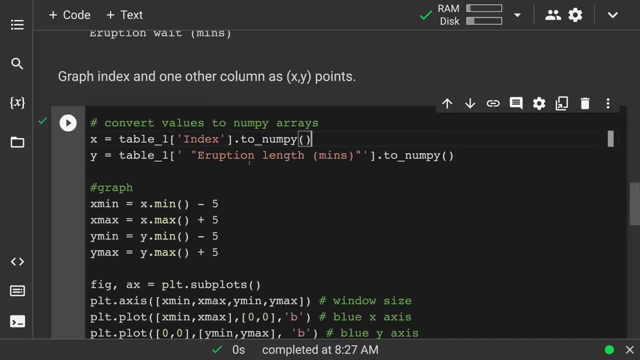 or i can do it for eruption wait times and i'd like to go back to the index again. x is 1, y is 79, x is 2, y is 54. so i just graphed it for that first one and we can go back and 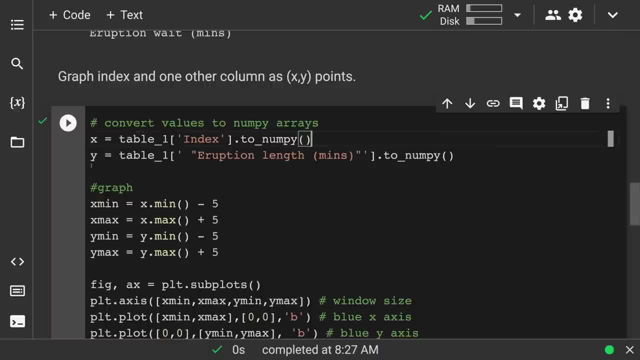 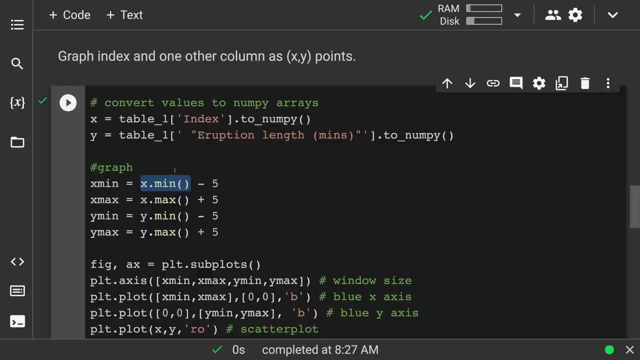 do that for the second one also, if you wanted to. so we have x and y. because they're numpy arrays, i can call that function x, dot, min and this. you know if, if you haven't really looked at like the entire table, this just might be a good way. i'll just take the minimum value minus five, because it's just a little. 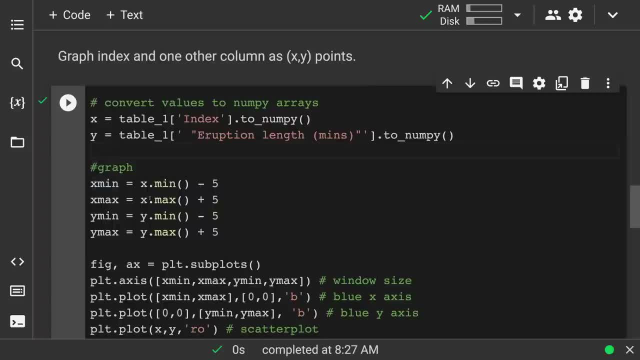 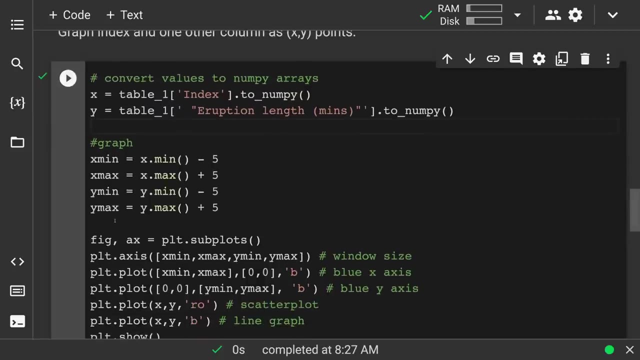 bit of a buffer on the edge and store that as x min, x max. same thing plus five a little bit of a buffer. y min, y max. and store that as x min, x max, same thing plus five a little bit of a buffer. so this goes back to things we were doing a while ago with graphing: set my x min, x max. 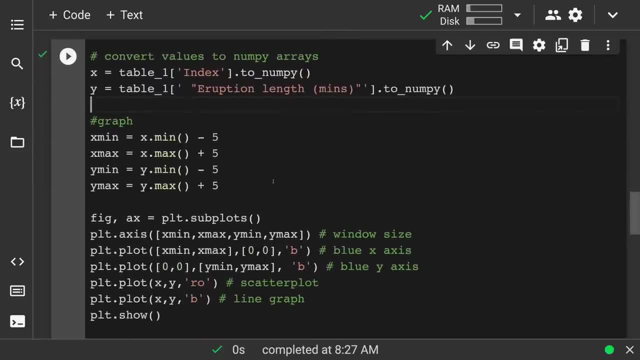 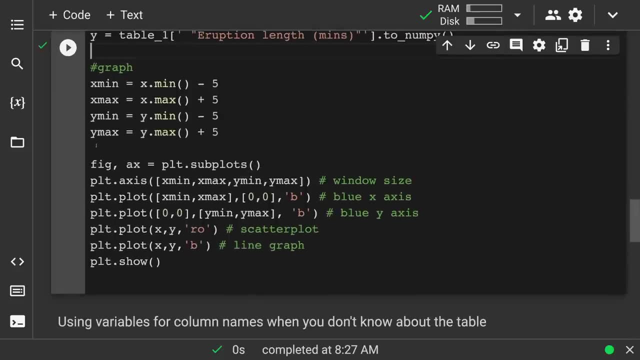 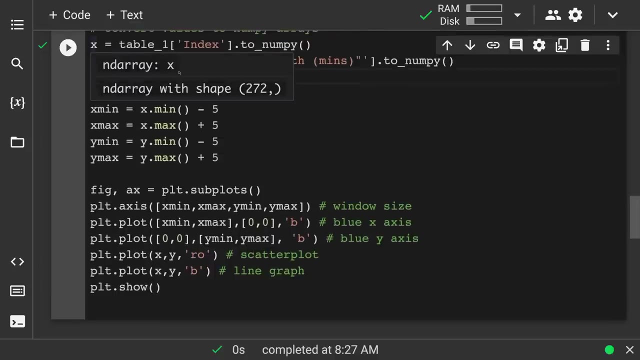 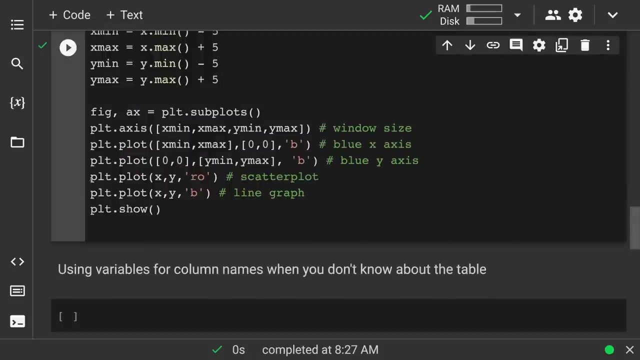 and each of these. now notice, i don't have some of the things we were doing in other other units. we were defining the points here, but i already have my x and y values defined as num numpy arrays. so when i graph, i can plot, i can plot them here. as you know, the x refers to that array, y refers to that array. 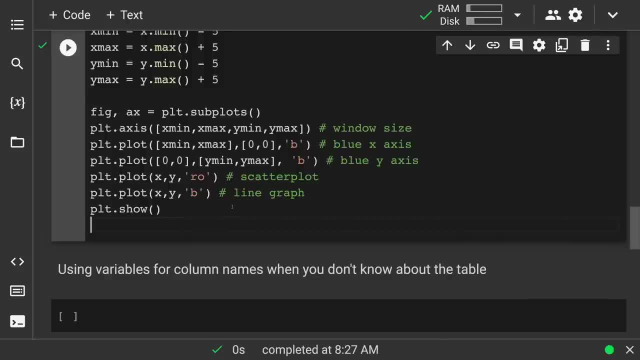 and i can do a scatter plot or a line graph. so i have these here as numpy arrays and i can do a scatter plot or a line graph and i can do a scatter plot or a line graph and i can do them as a scatter plot or a line graph. 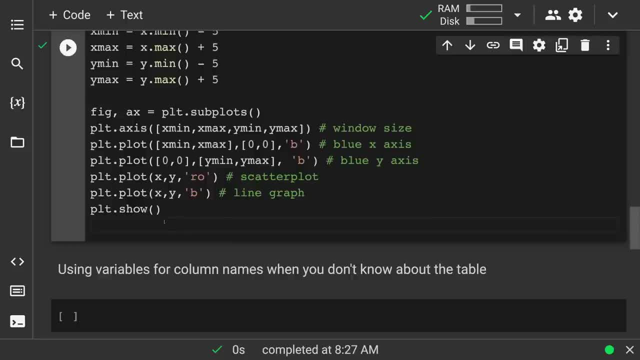 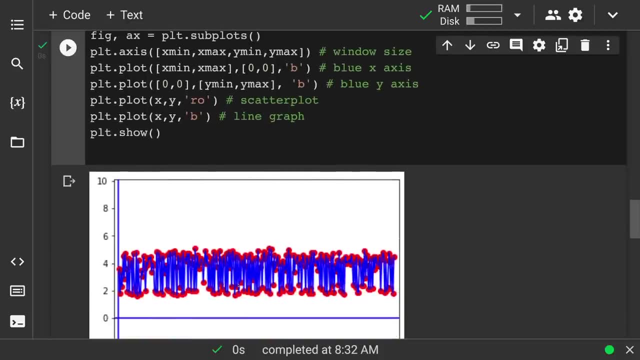 all right, let's see what this looks like now. i had it as both and looks like a huge mess. but one of the things i notice is: i don't want the line graph is probably not useful, so i'll just go. i'll just comment that out, right. 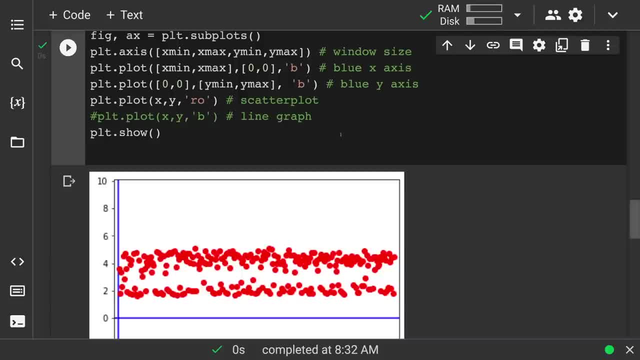 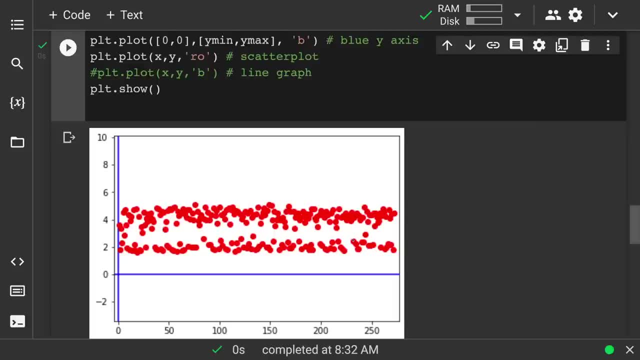 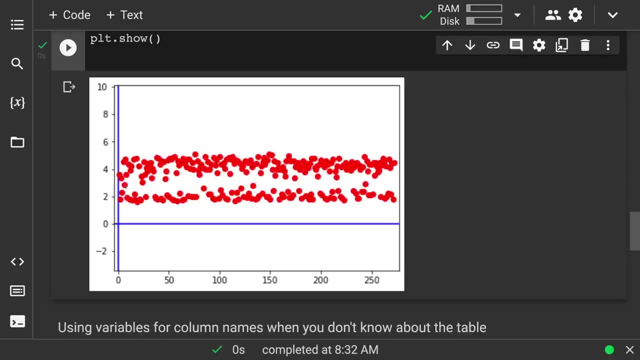 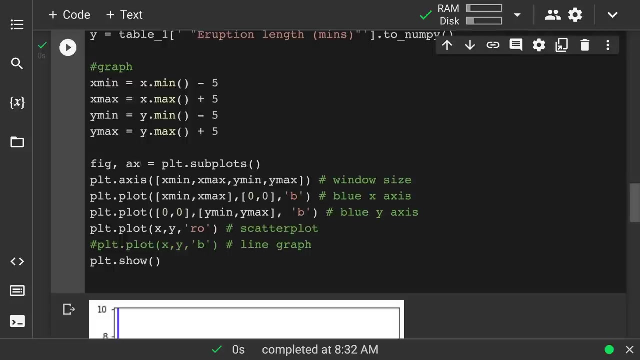 now and run it again and we see it seems to cluster. it's around here or around here. That's kind of interesting. What if I change my y value? Maybe I'll keep all these points, but what if I change this? so what I can do is my y minimum. and these are the things. this is what we want to do. 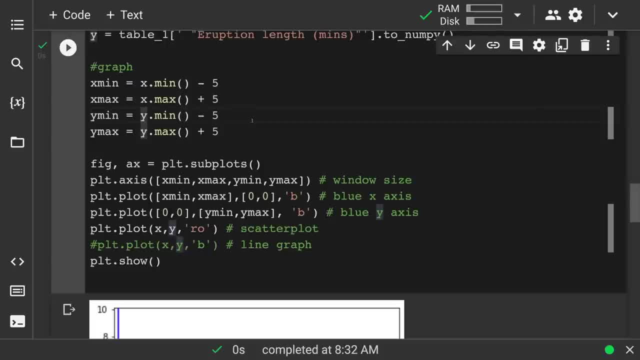 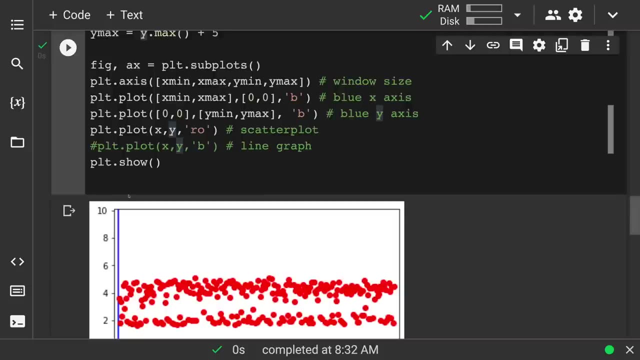 Now we know how to use your math graphing skills to look at this. You know how to get all this data into this graph. and this is now where we get to the analysis part. What can I do? I can look at this and say, all right, they're all less than six and they're all greater. 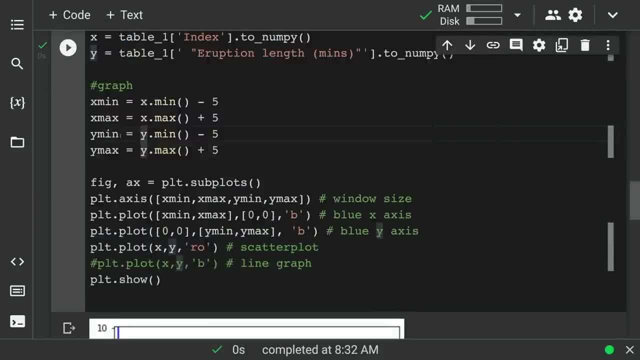 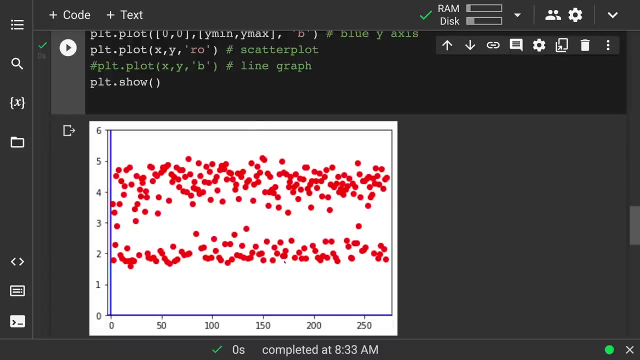 well, actually they're all greater than zero. so I can just make my y minimum zero And I'm just going to comment out the rest of this. and I can make my y maximum six and I'll just comment out the rest of that, and when we see that we might see. it seems. 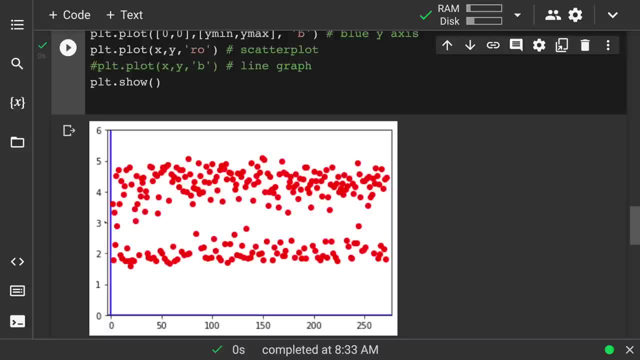 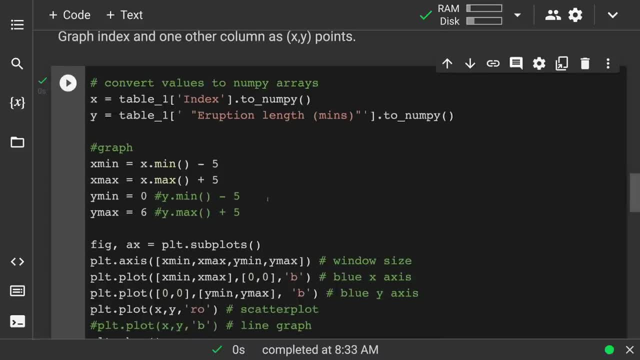 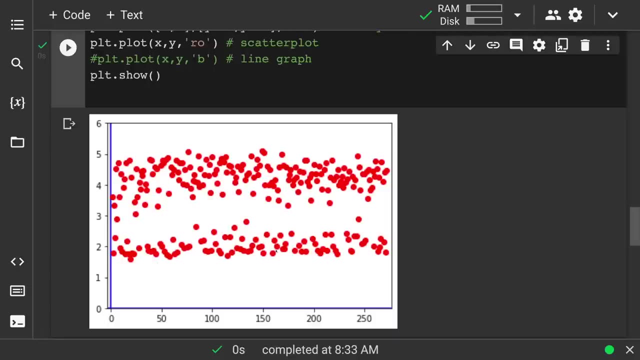 like it clusters For whatever reason. it's really rare for it to be around three. and remember, what are we graphing here We are graphing- Okay, We're graphing- the eruption length time, so it really seems to cluster around. oh, about two. 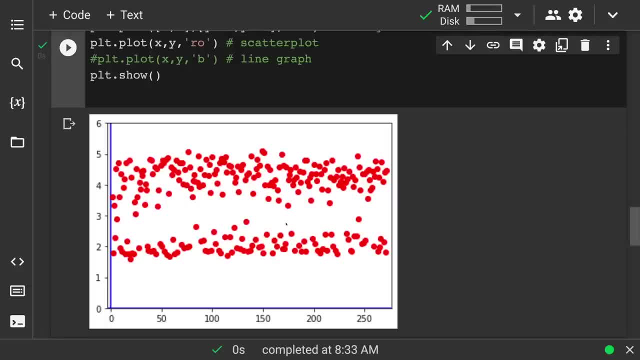 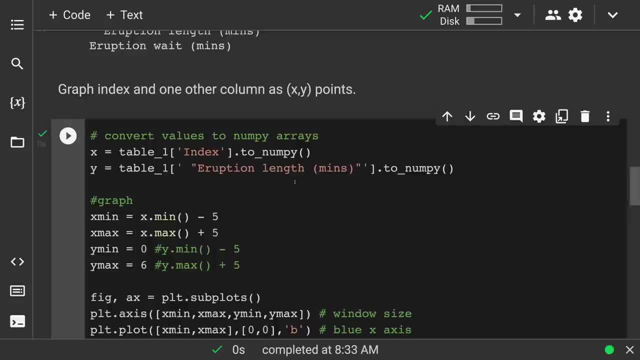 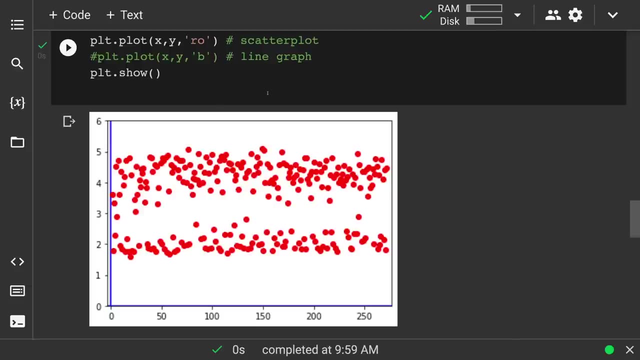 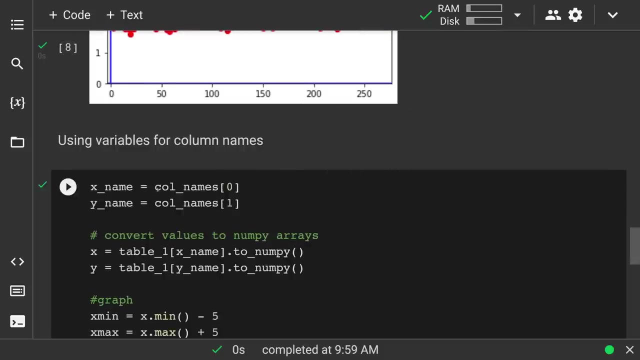 minutes or about four minutes. Yeah, interesting, So we can look at this and then one of the other things that we can do. now let's look at another twist on this. You can use variables for the column names. So remember, earlier we made column names, this array, so I can have column name zero. 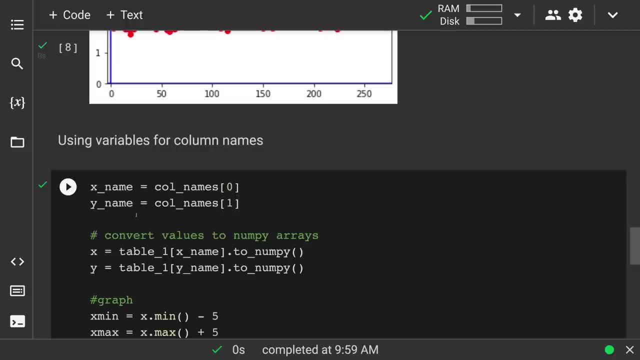 column names one, and that's my x name and my y name. I'll make these variables So that also depending on the actual names of your columns, doing that once might save you some typing, because then you can reuse that variable here. 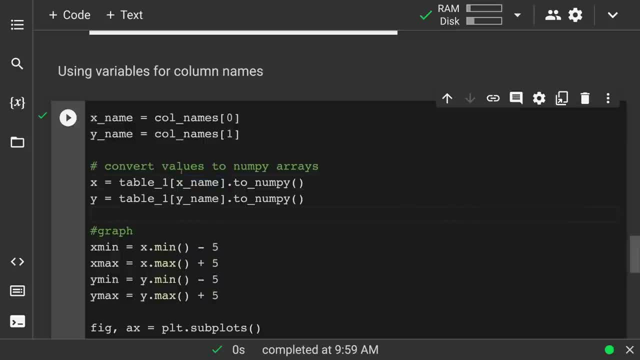 Just yeah, I don't have to do that, I don't have to worry about all the quotes every time. Now I have my x variable, is that column numpy? my y variable, that column, just like we were doing before. but again we're using that. 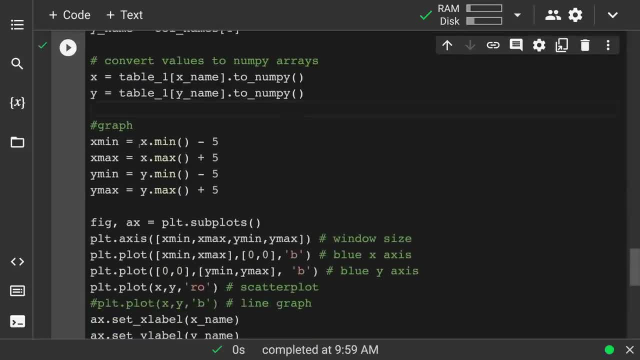 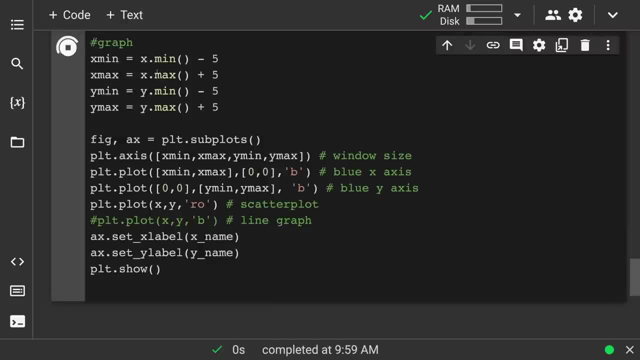 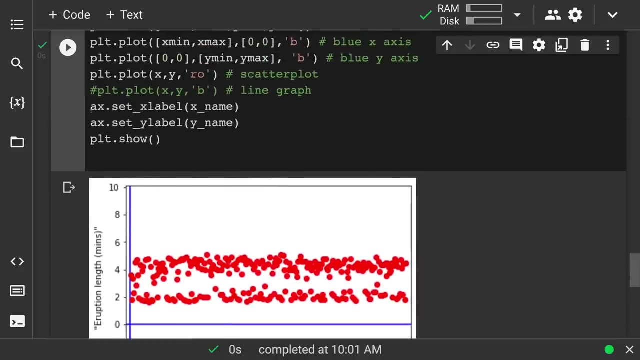 variable, save you some typing. I went back to this and we'll see why in a minute, and I just want to show you that that same scatter plot back to that. those original dimensions are there. But you see, using that as the column name, I can also set the labels for the graph. and again, 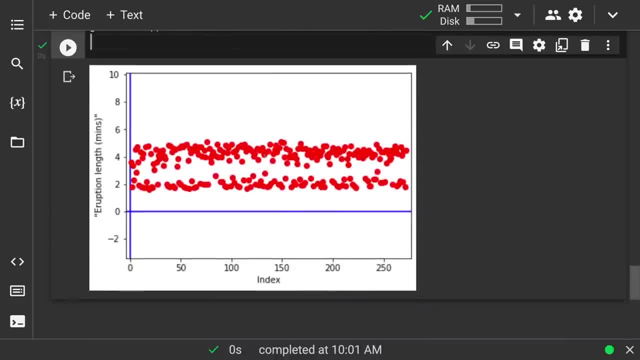 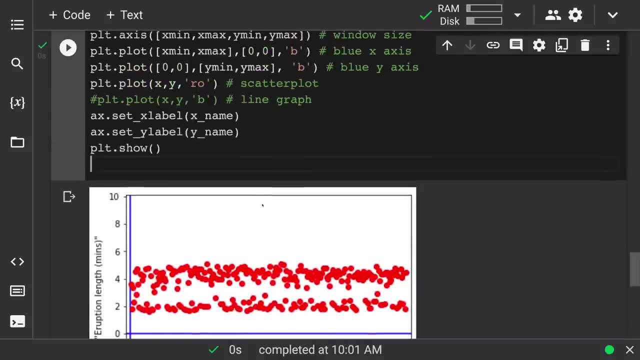 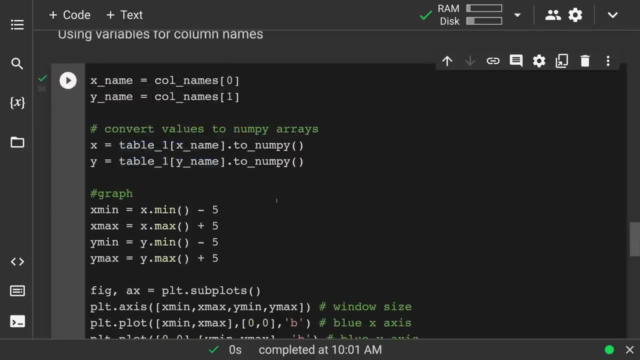 without having to rewrite. So now we have index and eruption length. There we go Then. if I wanted to talk about the eruption time or the erupt, the wait time, So all the things that we were doing, I can just change this. 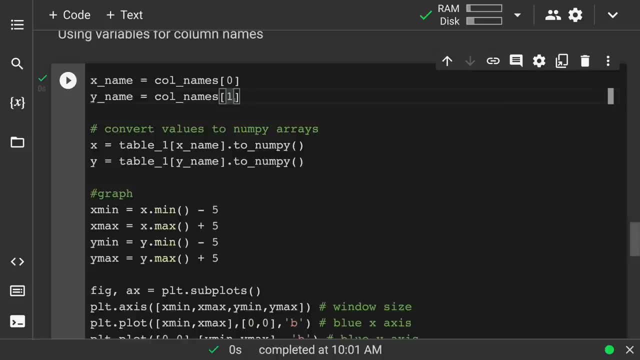 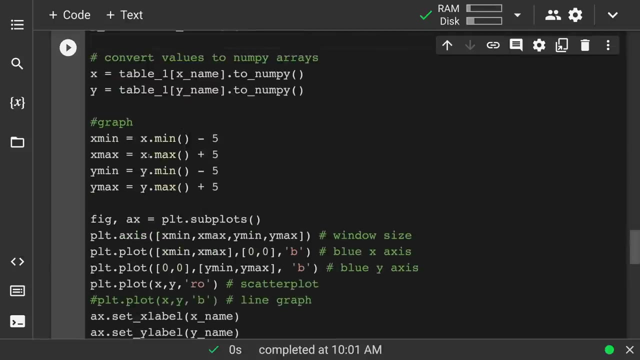 I still want the index, but then columns one was the eruption length. I'll change that to two. That was the wait time And now I have those names. Everything else stays the same And again going to different columns. that's why I like giving the dimensions of the graph based on that. 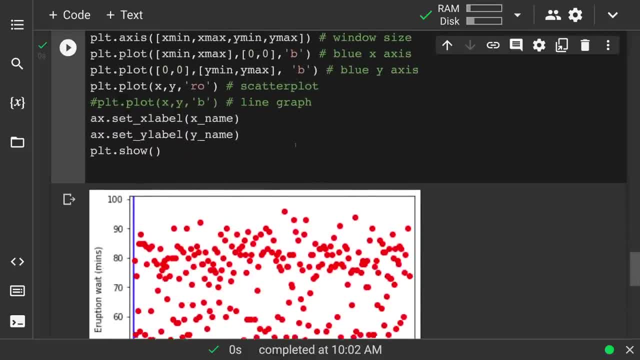 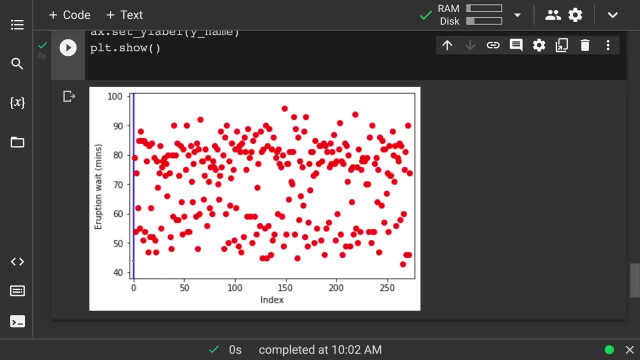 because these numbers are very different. I'll still have the same index because they did match, but instead of times between zero and five, I will have wait time in minutes: 40 minutes up to even almost 100 minutes. So we see that. 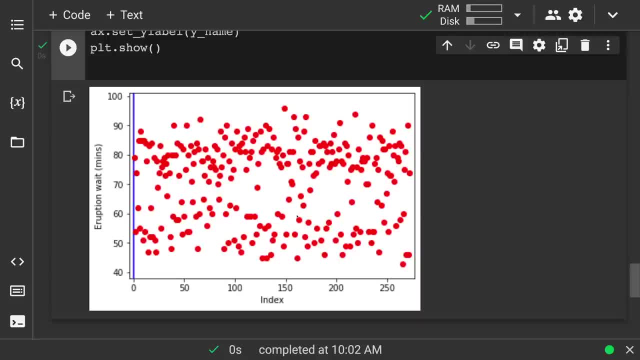 Now again, let's get to some analysis here. This looks like a mess. It looks like maybe I have this range of 40 minutes to more than 90 minutes, And this is key. Let's say this is in Yellowstone. Let's say you go to visit and you say, okay, how long should I have to wait? 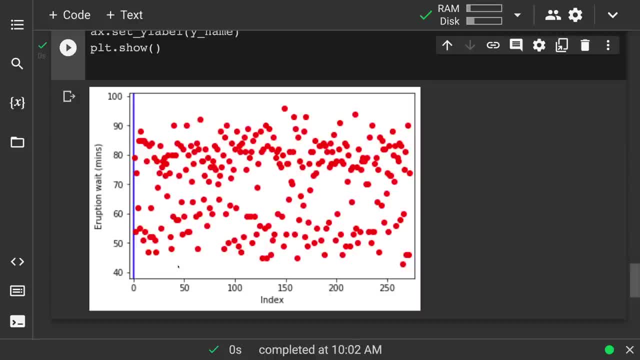 It just erupted. I want to go do other things. When should I come back? Well, should I come back in 40 minutes? Should I come back in 90 minutes? That's a huge range. It could keep you waiting there almost an hour. 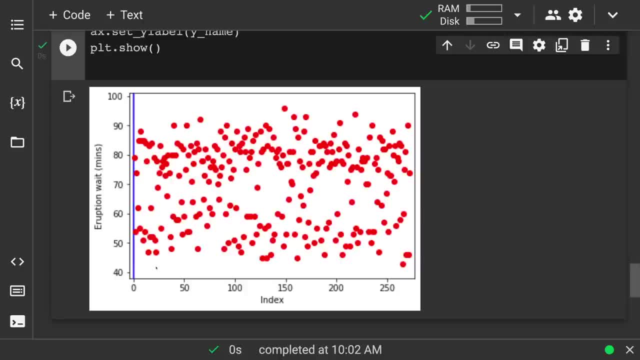 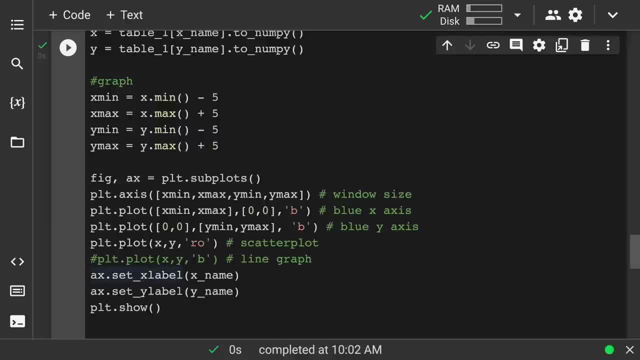 But let's start looking at other patterns. here Again, the default: I keep this index. I want to zoom in on some range here, So I'll go to that index. that X value, I'll keep the same minimum. But what if I change that maximum value instead of that plus five? 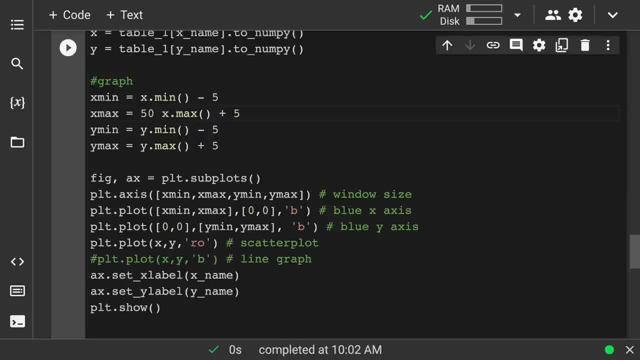 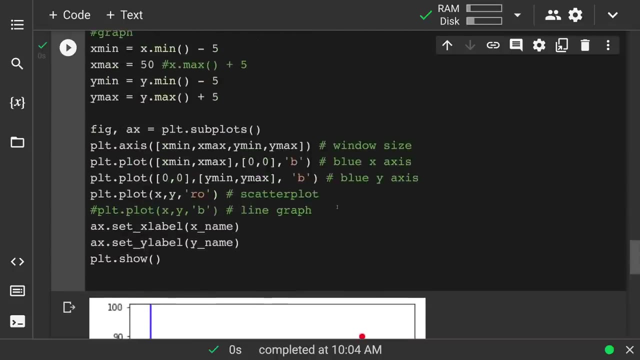 Maybe I'll make it like 50 and comment out the rest of this. So That's interesting. Um, I'm just going to run this again. Doesn't help you, but it spreads it out. You see, now, instead of a scatter plot, 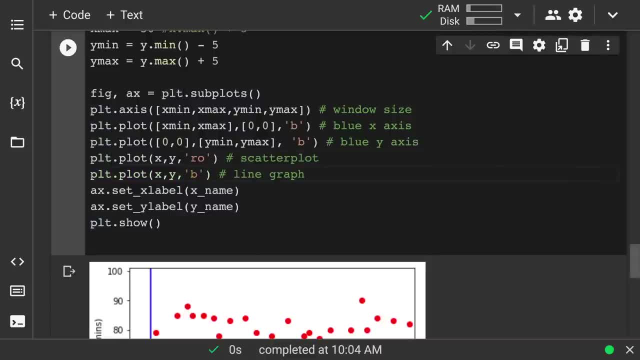 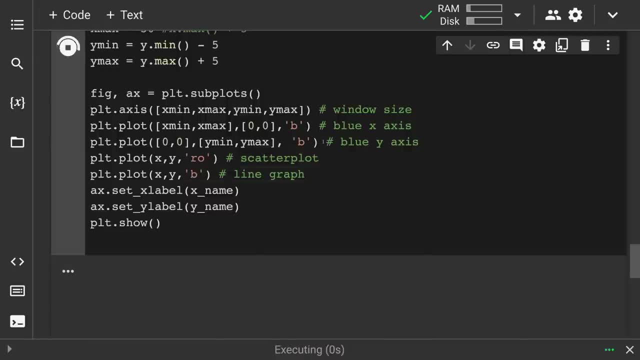 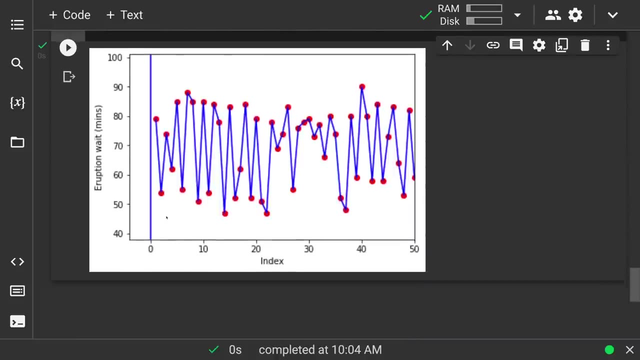 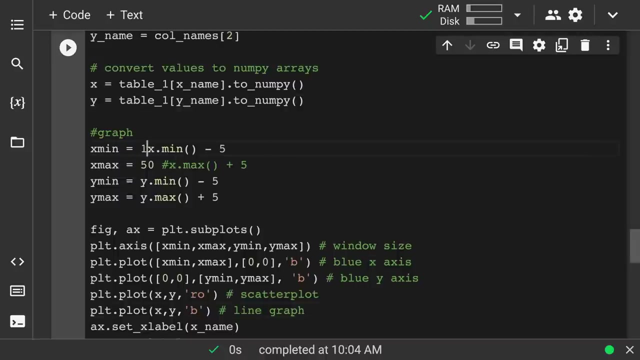 Actually I'll keep the scatter plot, cause that looks nice. but I'll also make it a line graph and I'll make the dots red and the line blue. So look at that And you see that just looks nice. Um, and if I don't, you know, there's my Y axis at zero. but if I don't want that, then I can just make my X, X minimum, you know one that way and comment that that way. 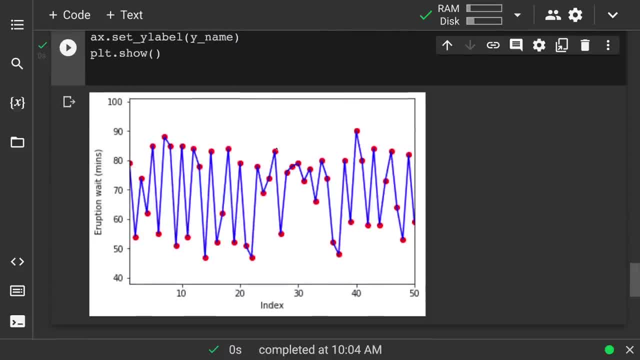 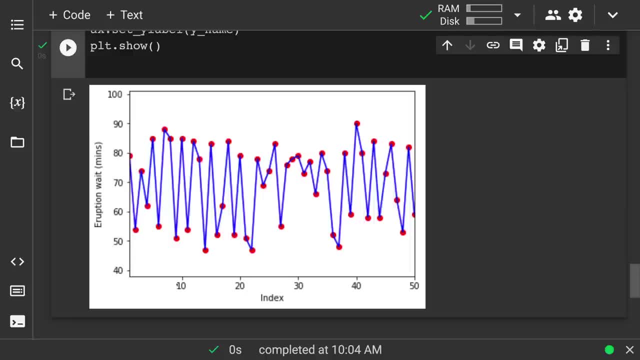 I don't even get distracted by that. There we go, So we take a look at this Now. besides seeing the scatter pot that was a mess, The line graph actually shows us some interesting things. with very few exceptions, If it was a shorter wait, like 50 minutes, the next one's a longer wait, closer to 90.. 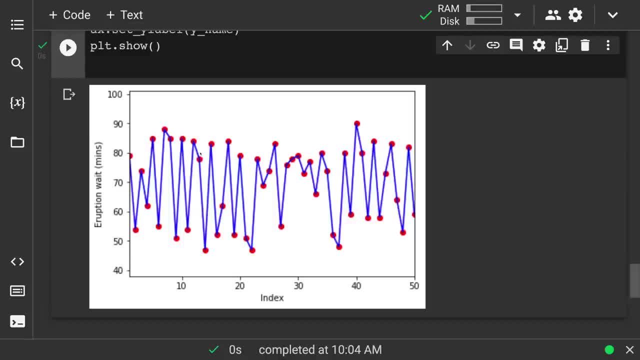 And then the next one's a shorter minute or shorter wait, longer wait. You see every so often you get one that it was another long wait, but we get a shorter wait, A longer wait, a shorter wait. you know, exception: longer wait- that happens most of the time. 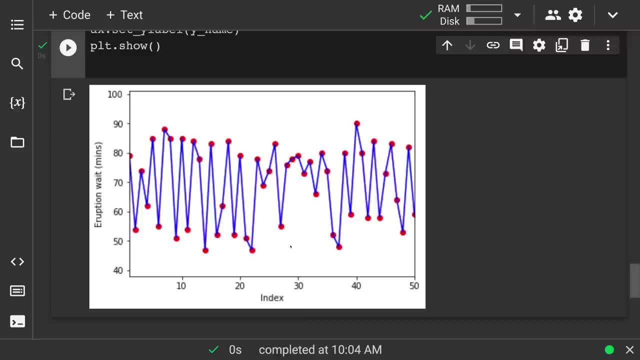 So what we can do is we could look at this and say, oh well, how long was it last time? And then, therefore, I can use that to predict, And we get that from you know, we get that from looking at the graph here. 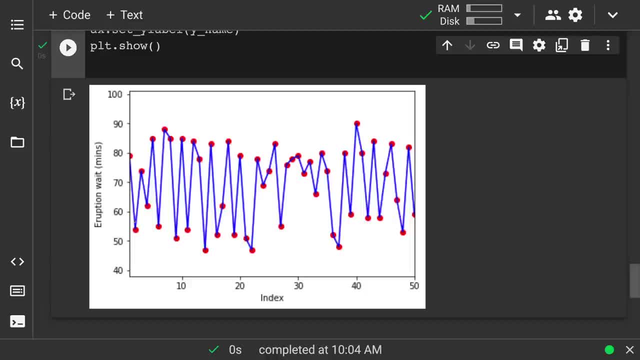 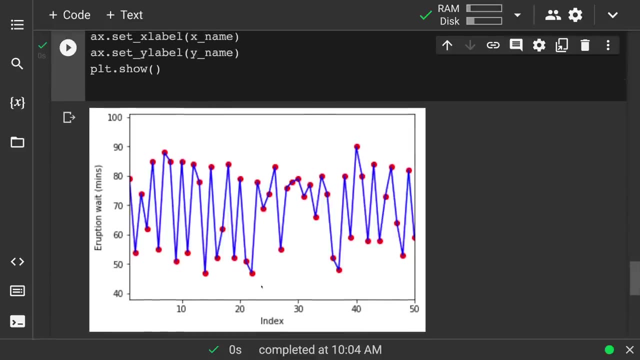 So, yeah, really interesting. I mean you could probably then Now connecting this to you know real time data science, Doing this, then we could graph, you know a certain amount of this and always, you know, have another table that always just updates you know when it erupted and how long. 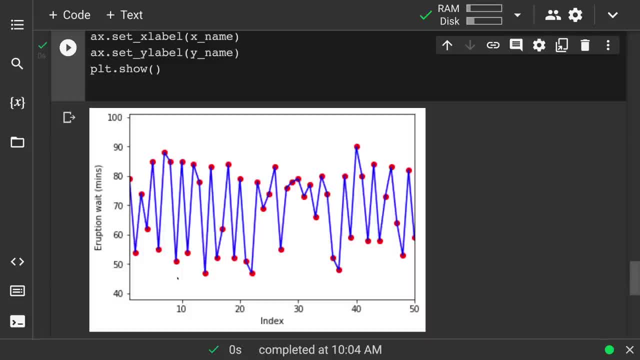 That would require somebody each time. you know, just you know. maybe even we could get this to clicking a button: OK, it erupted, It stopped erupting. and then do the calculations: What was the wait time, What was the eruption time? 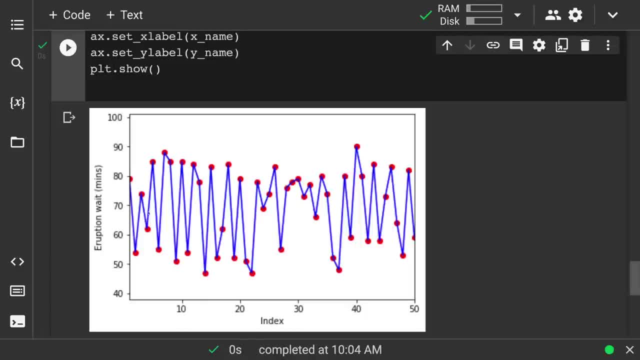 Add that new data and We could be looking at this and doing some sort of analysis to give people you know real time estimates of it just erupted. When can you expect the next eruption? and get it down even probably to some, like you know, confidence interval that. 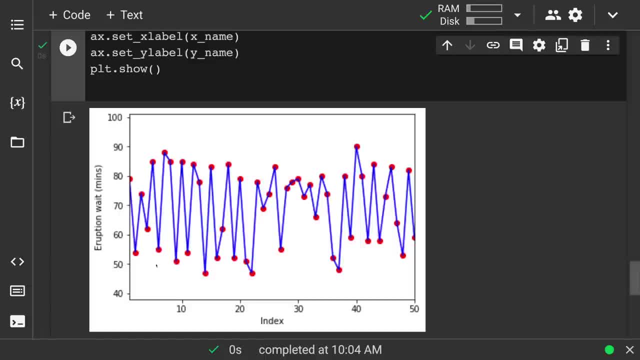 You know, the point is That you would want to be able to say instead of should I get there 50 minutes later or 90 minutes later, I want to be able to have, I don't know, like a few minutes. you know. if it just erupted and it was an 80 minute wait, then you know, would it be? you know 50 minutes, so you get some range, you know when to show back up and you know you don't have to wait too long. 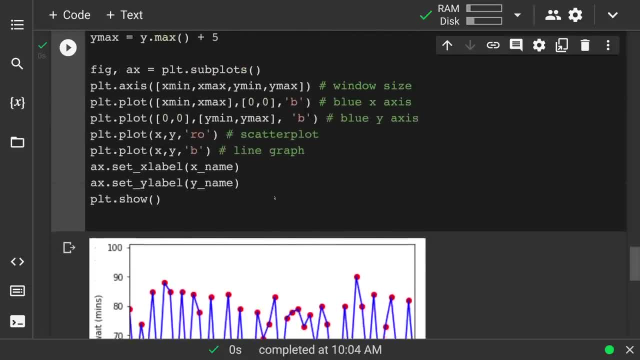 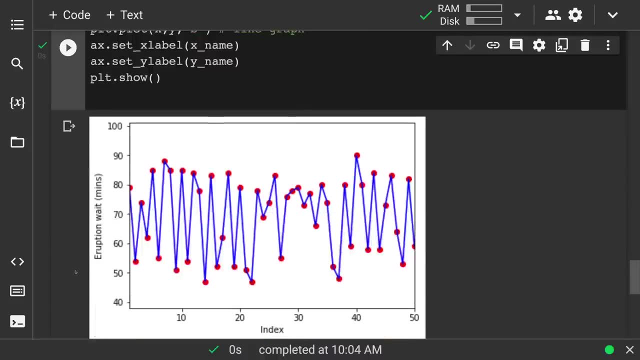 And that's really what we want to get this down to. We want to look at these patterns And be able to then, you know, predict the next one. you know that's really the goal. you know, if I go to here and I want to be able to predict and say, oh all, right, at 50, that was a wait time of 60 minutes. 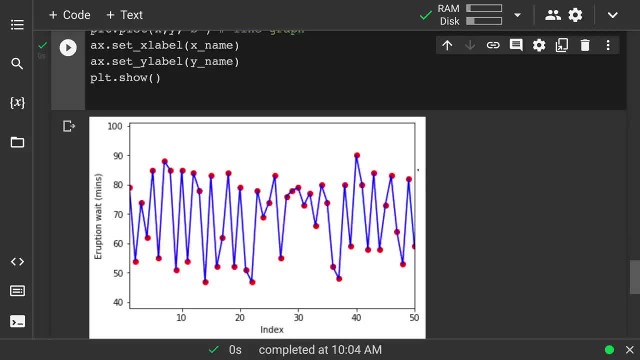 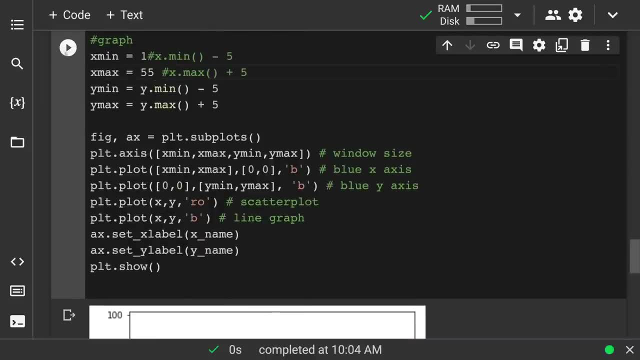 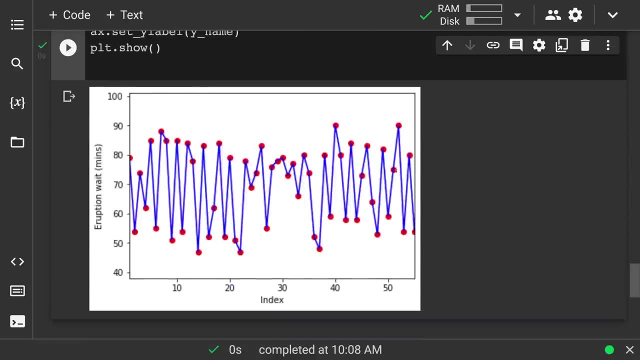 So I'm going to just predict that the next wait time is going to be more than 80. And if we really want, we can just change this to like 55. So with the wait time of 50 minutes, then the next one wasn't quite 80. 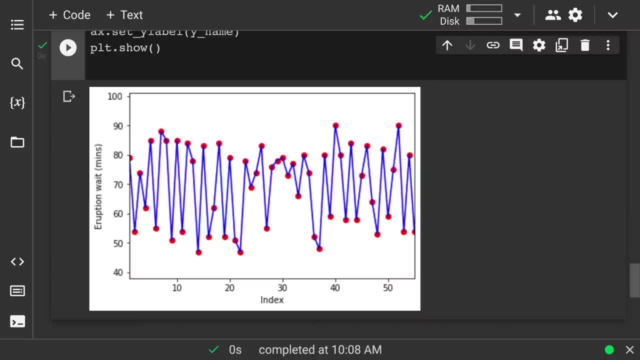 And so that's like your range of. well, I wouldn't go, I wouldn't wait more than 80 minutes, I might wait almost 80, and it'll show up. So there we go, Because remember the other graph, the eruption time it's, you know, three to five minutes. 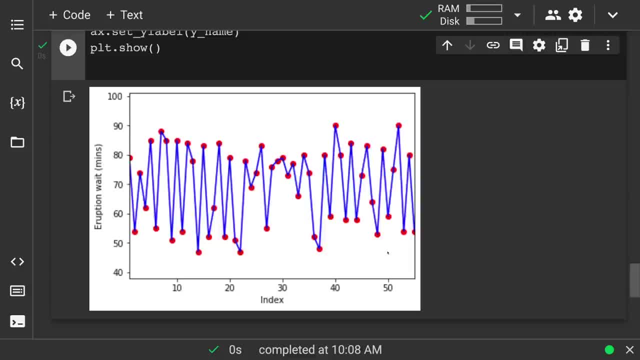 Or you know two minutes And it could be two minutes and you missed it. It could be five minutes. That's not even that long, So you don't want to be. you know five minutes late, You're going to miss it all. 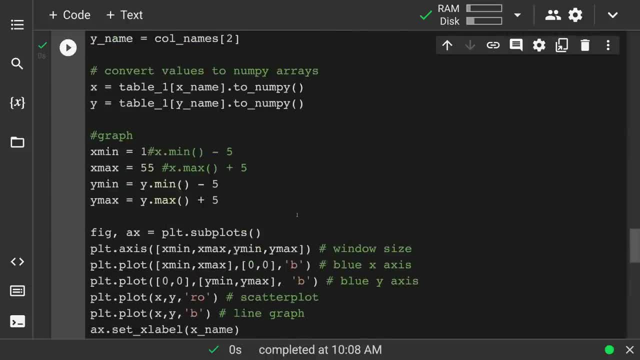 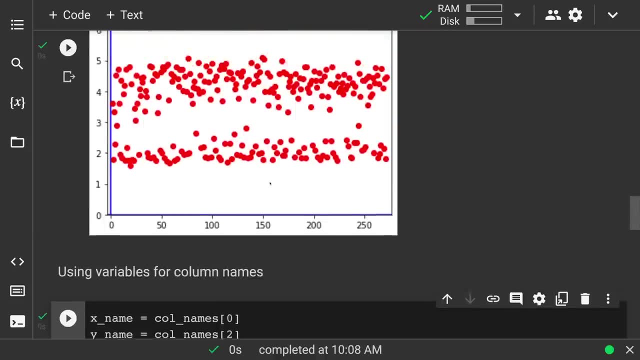 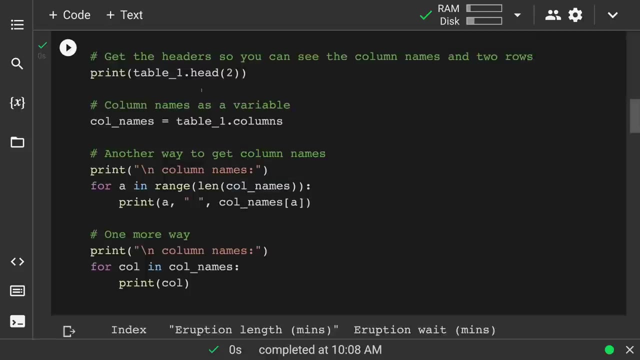 So yeah, just interesting, We can use this to predict. And again, looking at the math of it, we have, you know, once you have those column names. So once we have we get that table. Once you have that table and we get table one dot columns, you have those column names. 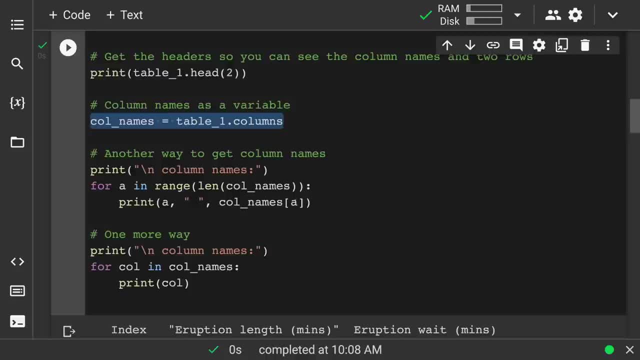 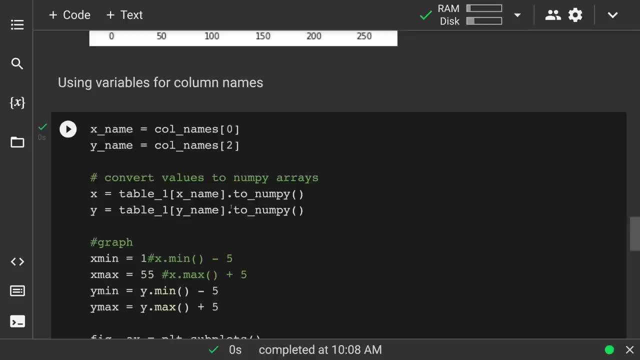 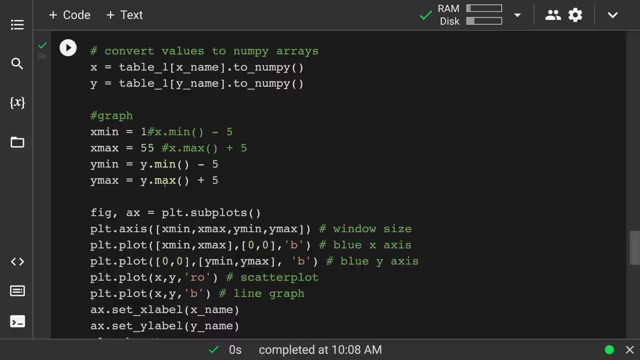 And then we can do other things with that, whatever we want. You know number them, you know just loop through them, or then pick certain ones And I'll use that as my X and Y. So that's the advantage of then having the graph: minimum, maximum. 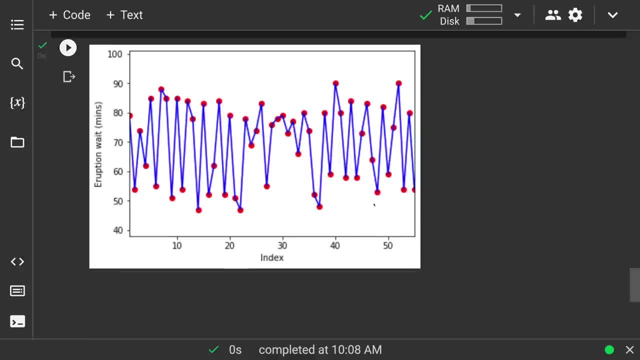 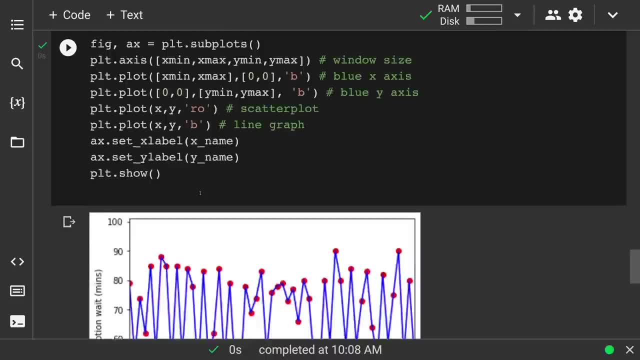 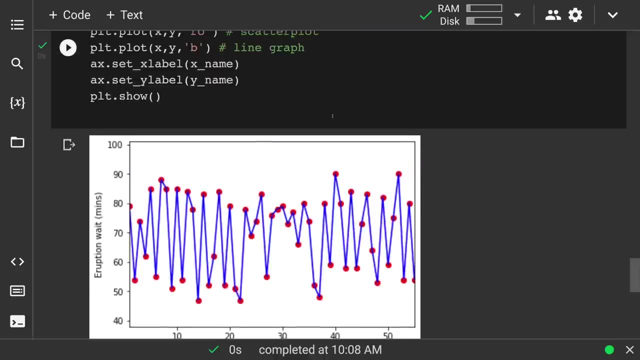 We can try this because we want to Make this template that you're going to have this and maybe certain things you can comment out and certain things you keep in. certain things you modify just a little bit. that what you can use the same code for whatever graph you have, you know, whatever table you have. 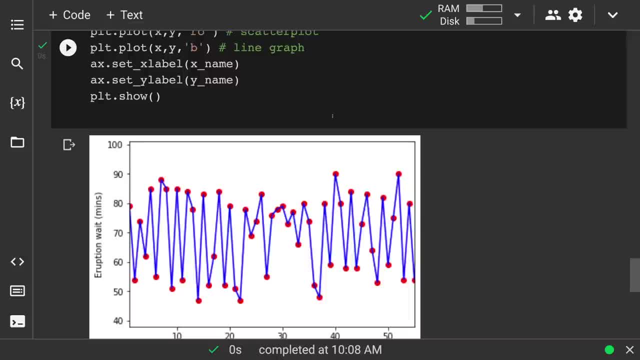 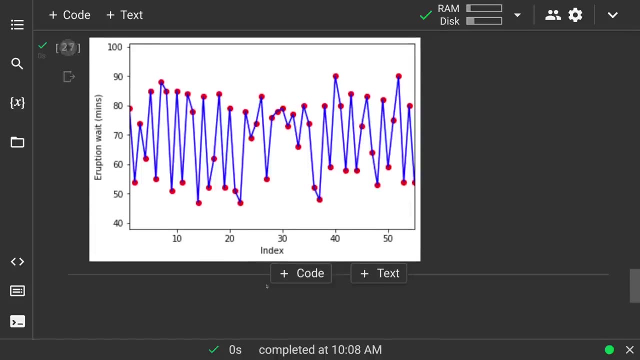 This is a good start. You start getting some analysis, What, what am I trying to compare, What am I trying to graph, And then, as you get into it, then you can modify. You know, you can always then copy all of this. and then you know, do in here, then copy all this, do a new code, sell some text to give you know yourself, or whoever read this, some some notes on what's going on in this code cell. 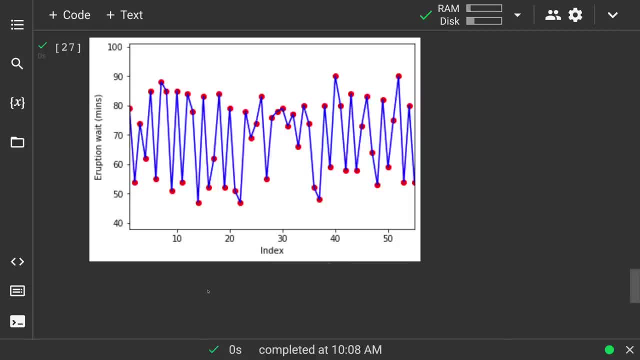 And you know that that's the beauty of the Colab notebooks. You know you don't have to like, you can delete things and retry things or you can keep that and then just you know, oh, this is, this is interesting. 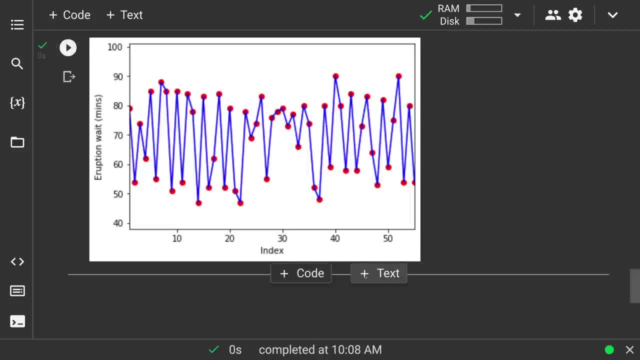 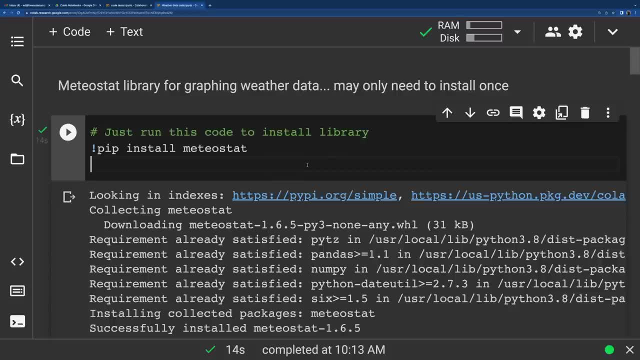 Information, Keep that and then just do a new code, cell or new text And you know let's do the next, next analysis. So here's another way to get data into Colab and then graph it, This particular library, so not a CSV but the full library- Meteostat. it's a lot of weather data. 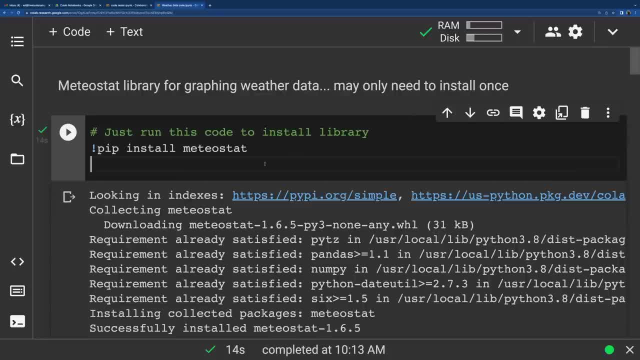 So, yes, may install. need to only install once. right, Once per one runtime. And I just have this as its own cell. There you go. PIP install Meteostat to install the library. doing that, I mean, this actually might take almost 30 seconds. 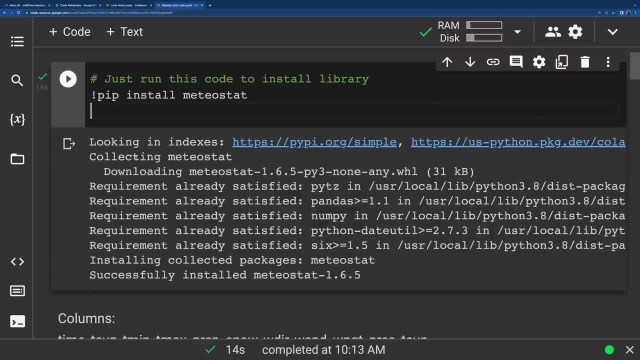 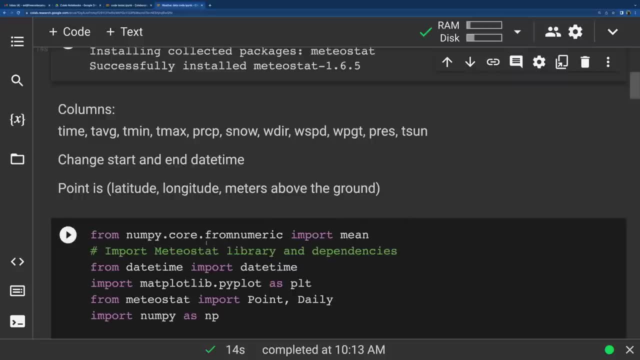 So sometimes that seems like forever. So I already did that And here we go, Successfully installed, And then we go on to the next one And for your own organization or anybody else working with this, you put put in some text areas here. 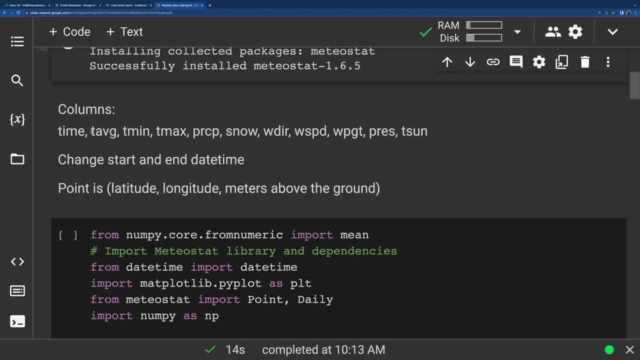 So now I know, and it reminds me what columns I have in this library. So time and all the other, these other T's are temperature: average temperature, minimum temp. maximum temperature, the amount of precipitation, amount of snow, wind direction, wind speed, the pressure. 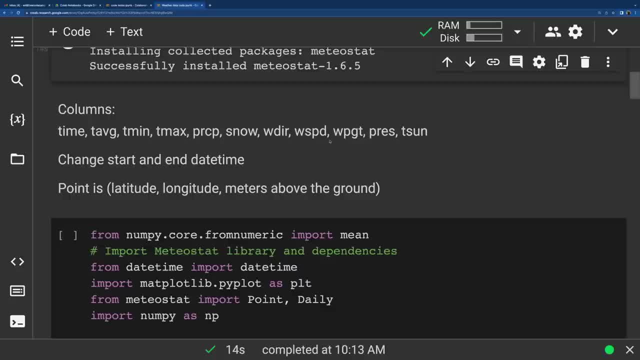 So average air pressure, air pressure, The wind gusts. So after wind speed we have wind gusts, air pressure, And the last one is time in the sun. So you know how many minutes of sunlight would you get. 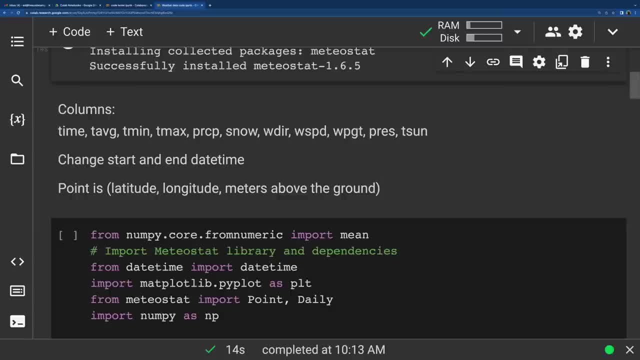 And these are really good. I pick these because it might be useful. You know you could things like wind speed, you know. plan your wind turbines and where to put them Time in the sun. Plan for your solar panels and where to put them. 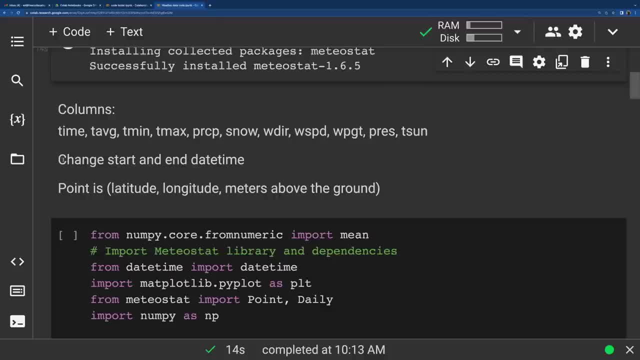 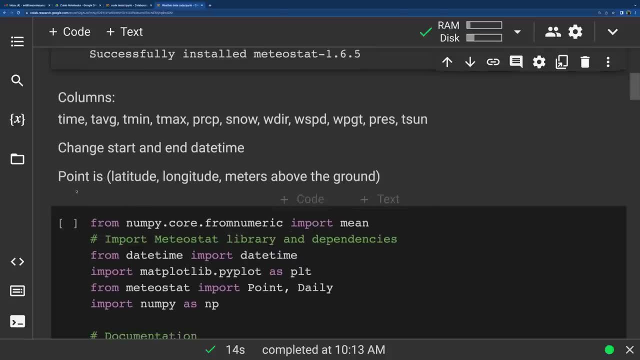 So I have these to remind me, and then the reminder change starting and date time And you know point, We're going to use this a lot. So what arguments is this expecting Point? latitude, longitude meters above the ground. 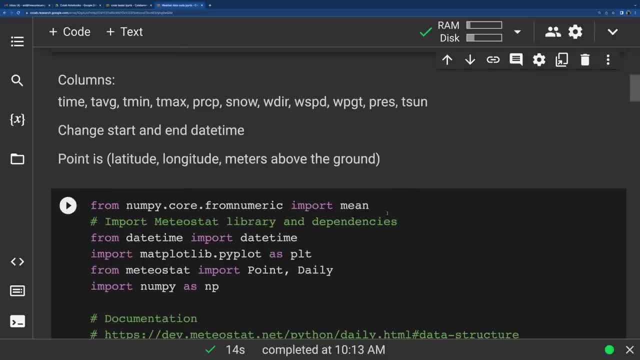 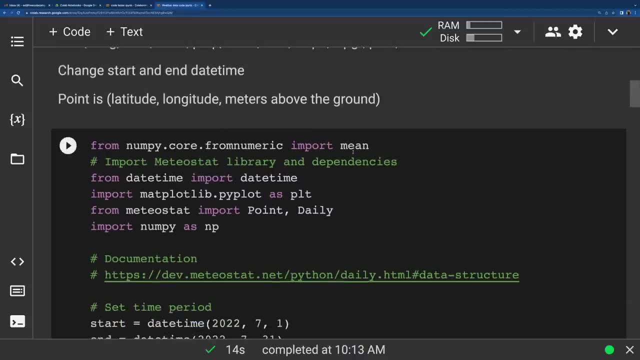 So now we have these notes, you know, Maybe you set this up for yourself and you don't. You use it for a while and then you forget. you know what you can, what variables you can use. So all this, you know, we can just keep this same. 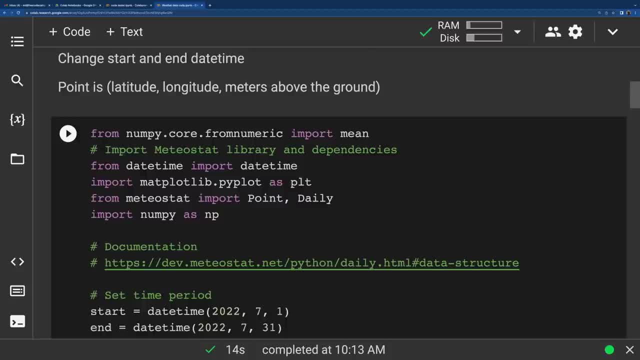 I just have the notes here because you have from NumPy We're going to import, mean because we're going to use that, And then the rest of these are from, you know, the Mediostat library. We definitely want date time plot. 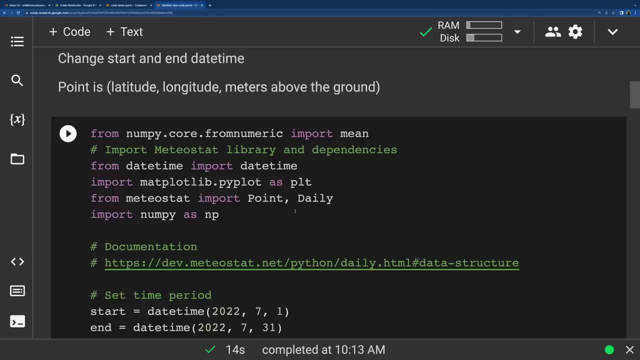 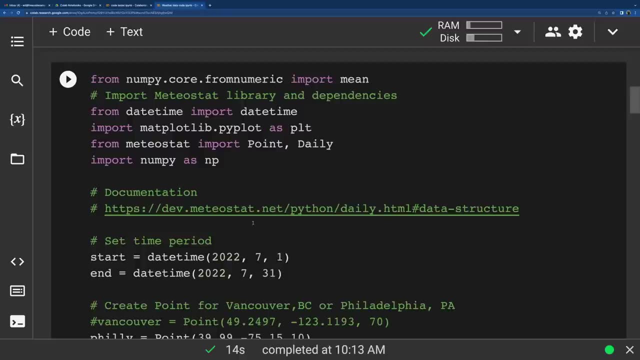 And for Mediostat, we're going to just import These couple of things Also. it's just, it's useful, but the documentation- and you know that here's the website where all the documentation is, you know, put that in there as a comment. 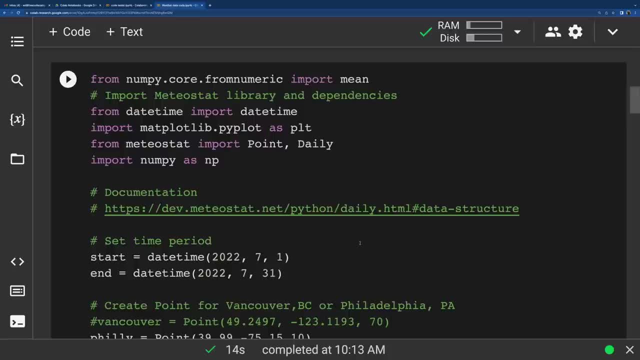 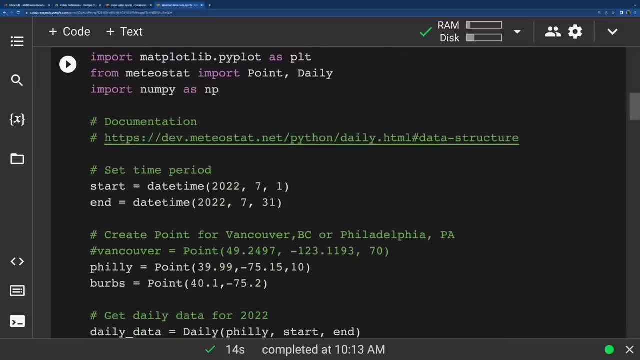 Again, just like the other notes for yourself or for other people. Good to keep track of these things. So now we know what we're expecting, We can set the time period, And what I wanted to do is I just picked, you know, sometime, you know, one month in the summer. 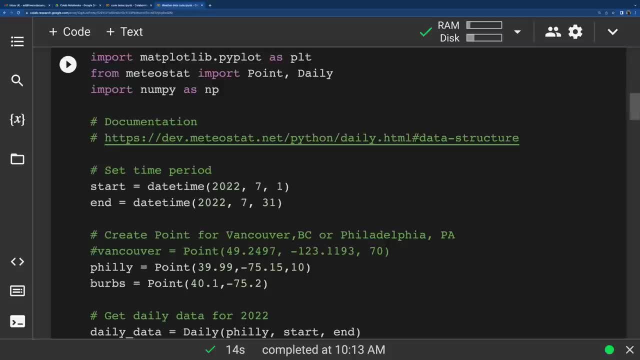 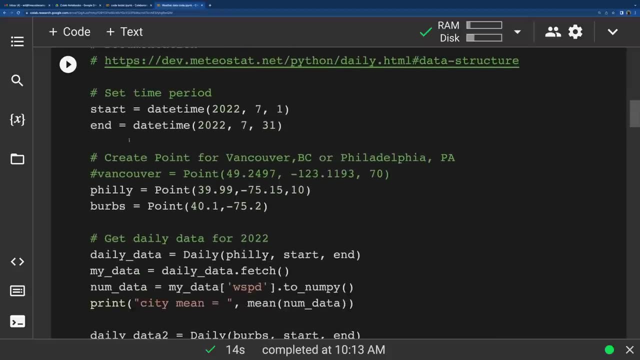 Start and end. So I have eight time There we go, Year, month day, year, month, start and end. And so the person who put out this one example online did this for Vancouver. So you know, I just commented that out and I did one for Philadelphia. 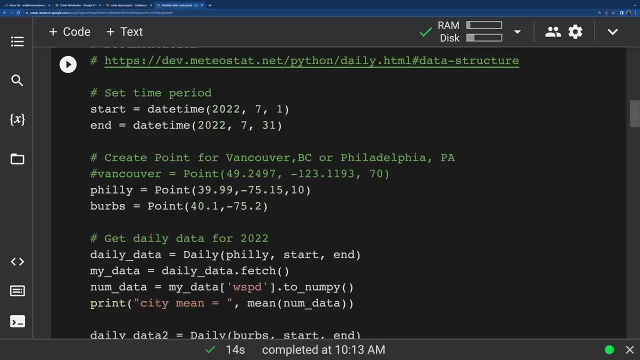 And I picked a random point in the middle of the city because it The if you want to click places and you get latitude and longitude, you get a lot of decimal places. So I just wanted to round it to two decimal places and see where you know, you know in Philadelphia in general, and then round it to two decimal places and see where we got. 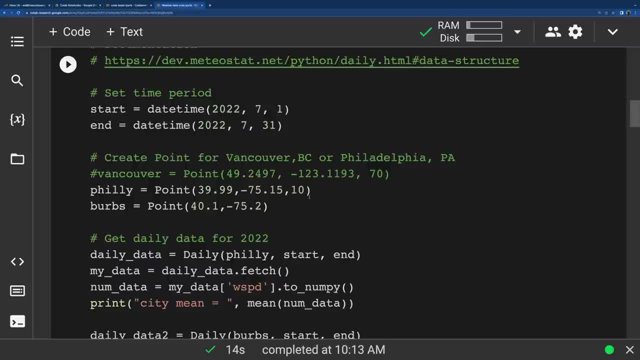 So it's some random street corner in the city, And remember that. third argument is how many meters above the ground. So I put ten, because this could be a wind turbine, you know, on top of a building And I wanted to compare this to somewhere in the suburbs. 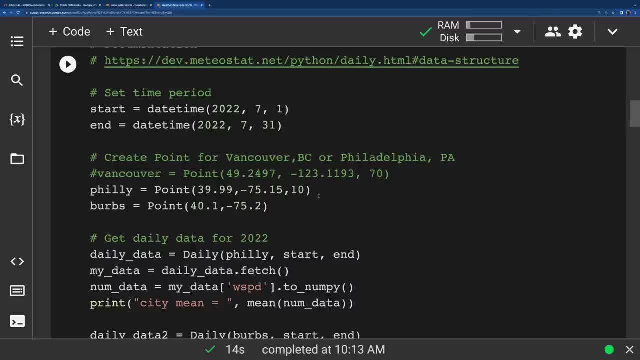 So, you know, are there closely packed buildings? Does that affect wind speed? Well, we're still talking ten meters above the ground. So this is in a residential neighborhood. that is probably above all the buildings. But I picked a point in the suburbs and I picked a point that seemed to be like a relatively open field as something to compare. 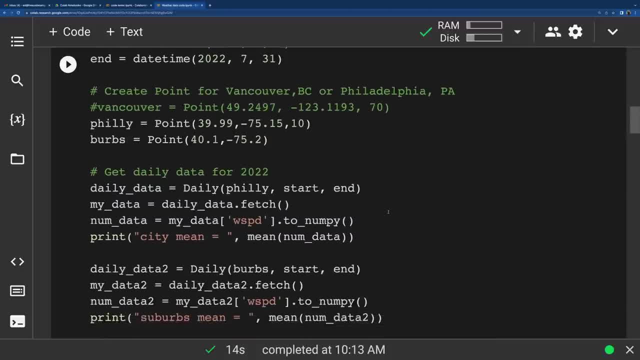 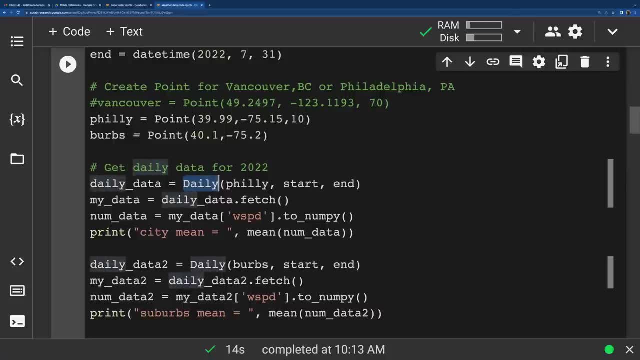 So now I have these two points and I can get this daily data, So daily, So that's the function in in Mediostat. And there we go, I get this particular point. You know, these are the arguments at that point, and then start time and end time. 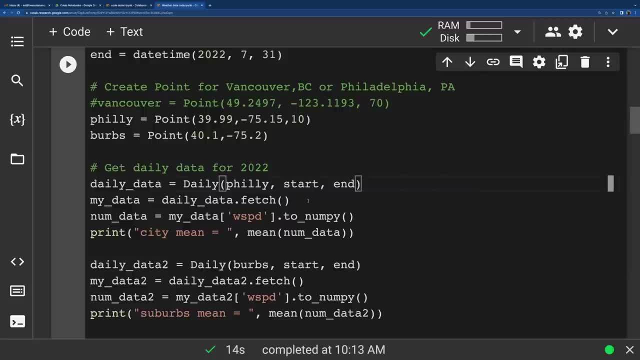 And then we go to this daily data, that fetch, and I'm going to store it as my data. Now we want to take this Um my data, And which one do I want? I want wind speed for this one And remember our function got to NumPy and I'm going to store that. 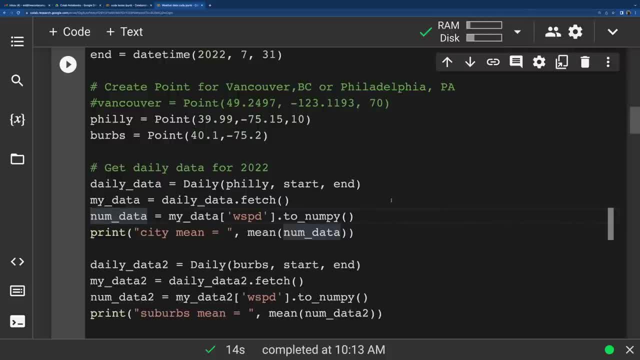 So now num data is my array and you see these layers that we want to do. This library requires this function here. I'll store that as a variable. Now that variable dot fetch, That's also from Mediostat. I'll store that. 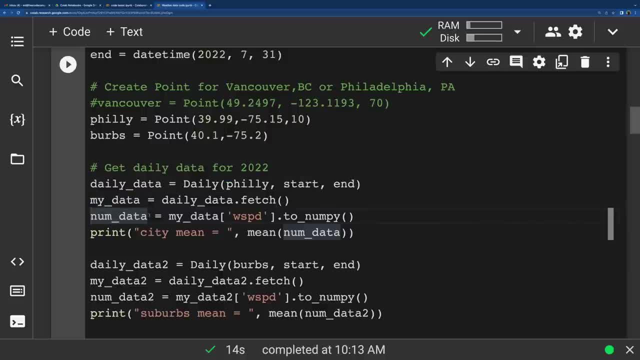 But then I that's not enough. It's a NumPy array, so I want to make that a number. I want to take that, calculate- you know wind speed, that column and make that a NumPy array. So I'll print that. you know city mean equals and I wanted to get the mean. 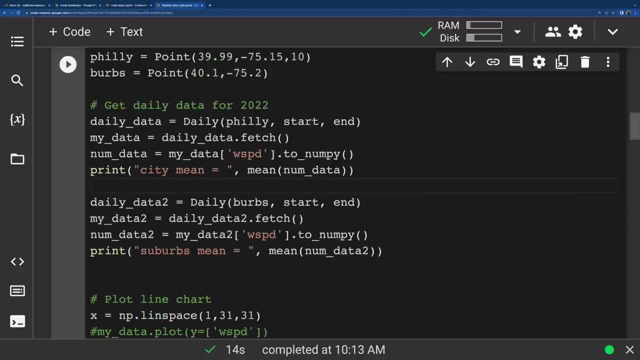 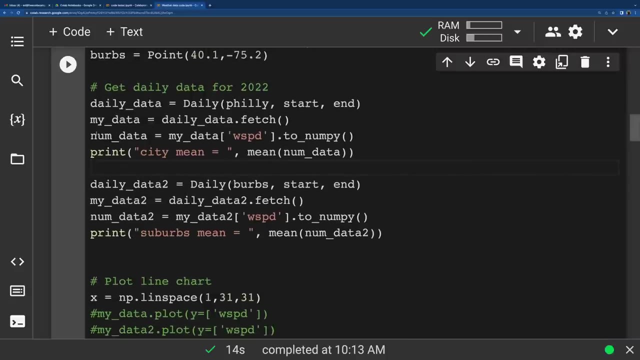 To compare. So now I have the second one. Again, I'll do the same thing that daily function: fetch the data, Convert it to a NumPy array And in this case I'll do the suburbs mean, But remember num data and num data two. 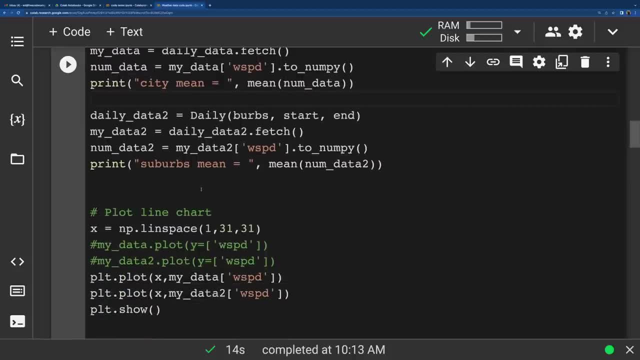 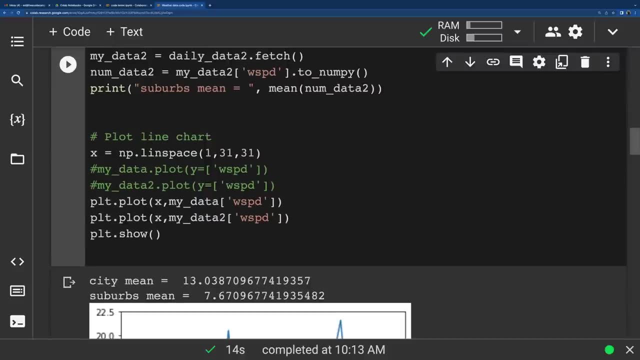 They're my two NumPy arrays So I can use them to plot, So we can plot the line, plot the line, There we go, And so I have this. you know these two things I have. you know The x value is: 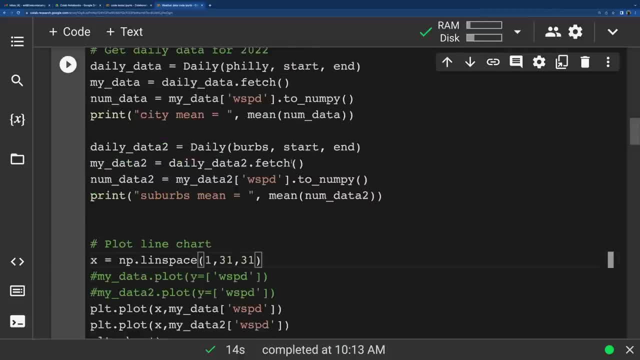 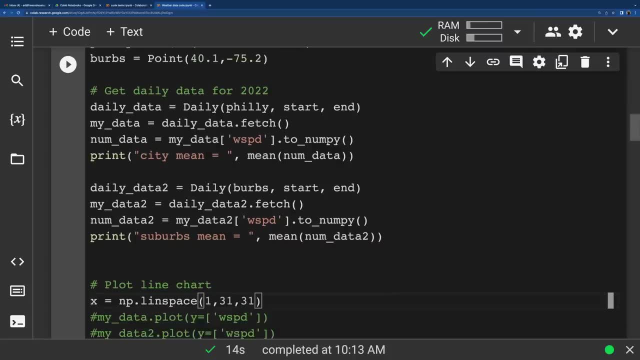 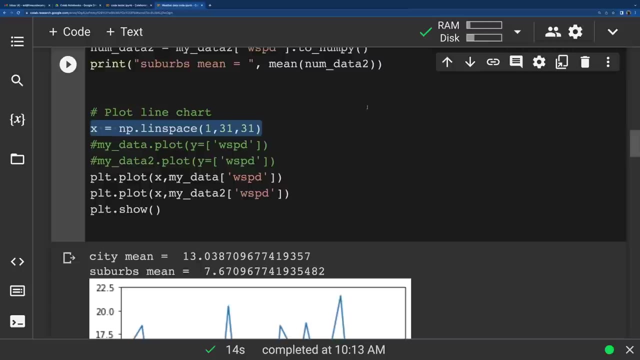 Since I know that I made my, Since I know that I made my start and end time. you know 30,. you know 30 days. I wanted to make the x value. There you go. Same thing, One to 31.. 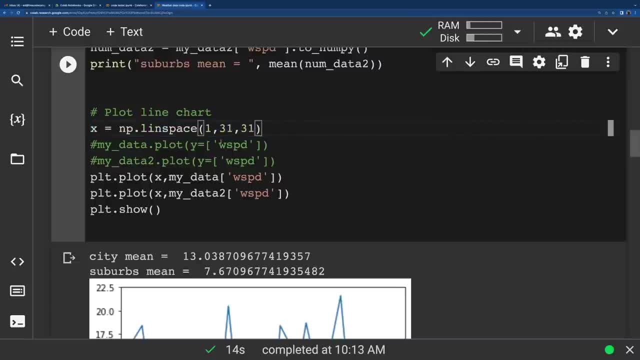 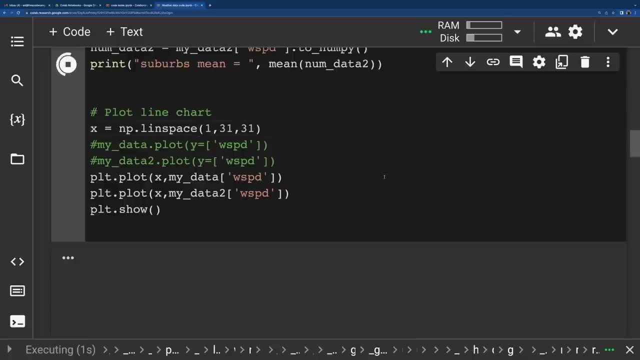 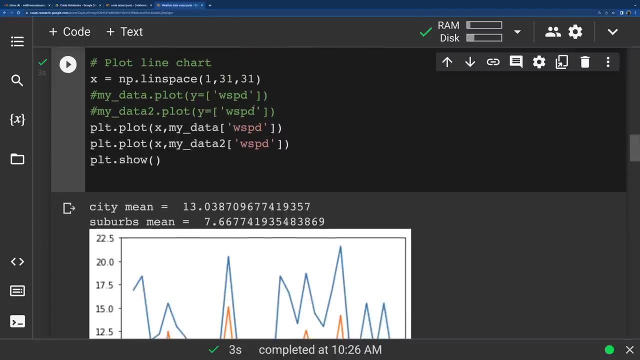 31 instances because it includes the first one. So there we go, And then I can plot these wind speed and run it All. right, Now I'll tell you why I have that commented out. I'll tell you now that I have these because this works like. I wanted to again connect it with. 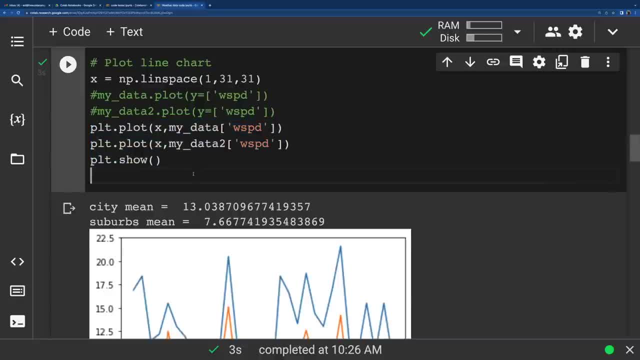 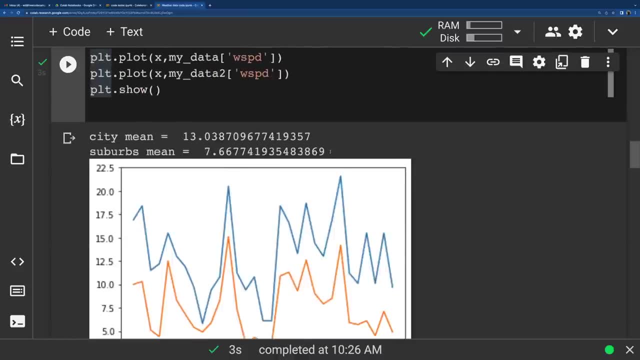 The same type of plot. you know matplot library that we use. I wanted to connect it to that same matplot library that we've been using and show you that that's what you can do. You know, get those arrays and plot them here. 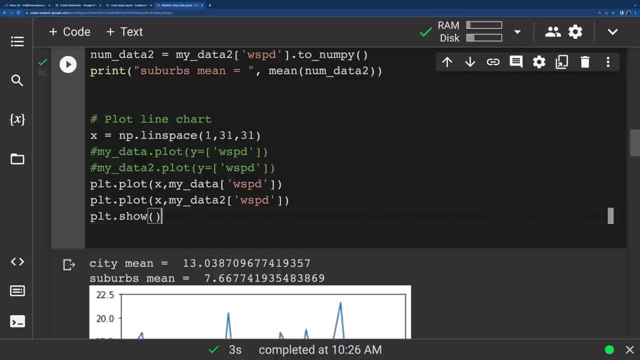 The plot that show. but I commented this out. This works also just a unique feature of this library. You can just take that my data dot plot And then in parentheses you know what the y value is. So these two work. So I just wanted to show you. I'll leave them in there. 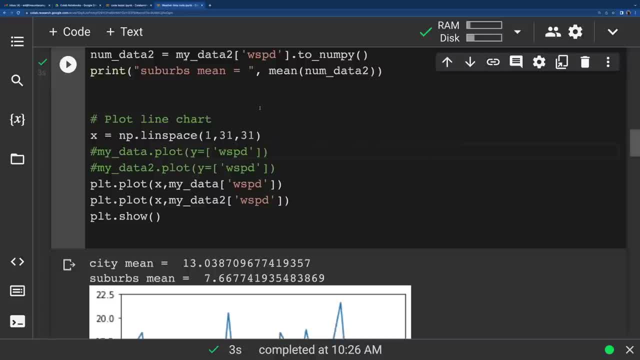 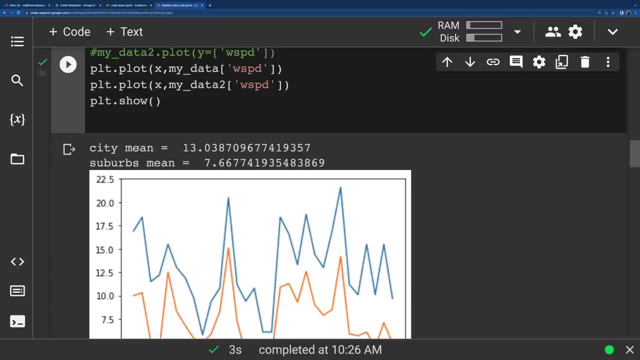 They work, but in order to connect this with the The same type of math and plotting we're using, I plotted them this way And so I had it calculate and then just display. you know, the city mean and suburbs mean. I could have rounded it, but 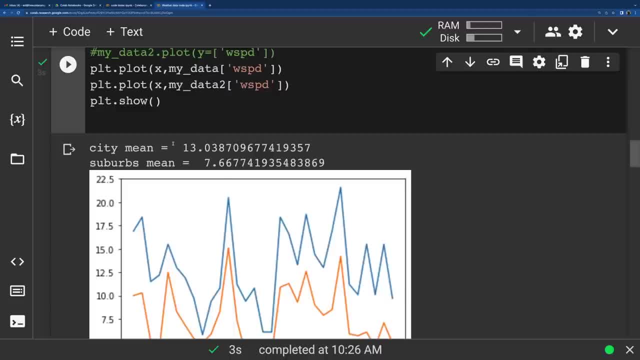 And, quite honestly, this is why we do data analysis. This totally surprised me. I really thought the average wind speed in this suburban area- that was like a relatively open field- would have been significantly higher, And it was definitely higher in the city. Yeah, interesting. 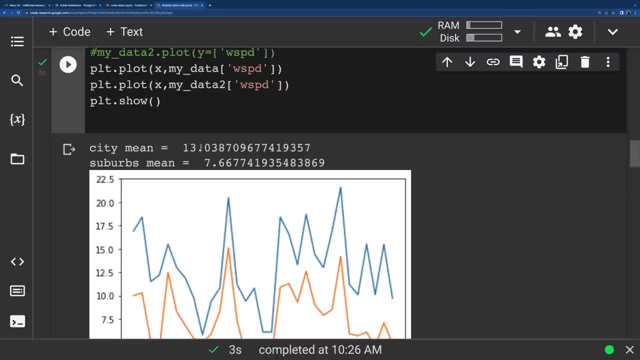 Maybe you know a little bit of a tunnel effect, Maybe there is some something going on with. you know the buildings. Maybe that wasn't high enough Also, at least in Philadelphia, that city, and if it's high enough that's a little bit closer to the river. 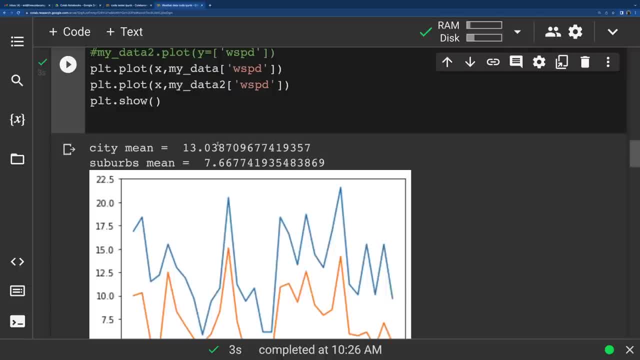 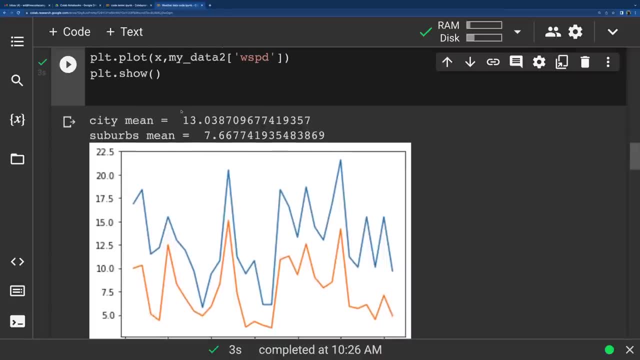 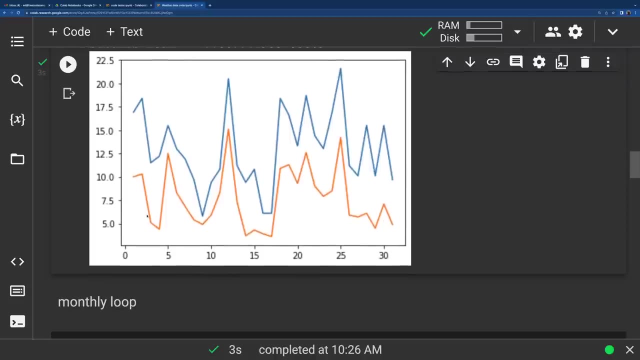 Delaware River is. you know, any river gives off a little bit more wind and this was a little bit closer, So that might have had an effect. but there we go. So then we See the mean, but beyond that we can see the tracking. you know day to day and you know there's still. these two points that I picked are not that far apart. 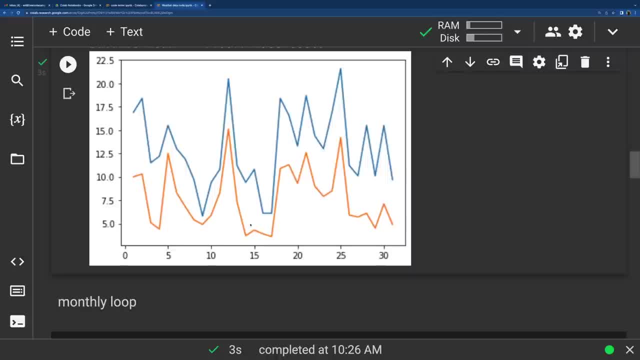 So it tracks there in the same area. The wind speeds go up and down, you know, in very similar patterns, but we see that not just the mean, but at every single point. that city location was higher. So there we go And 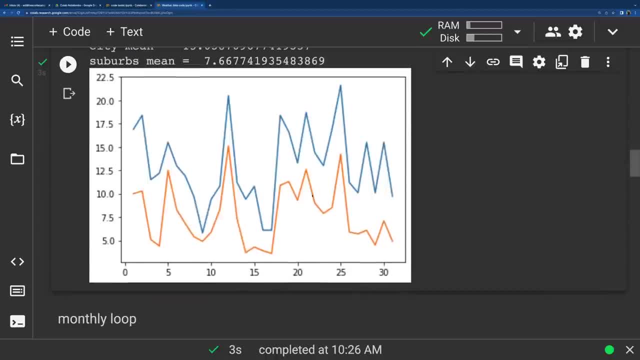 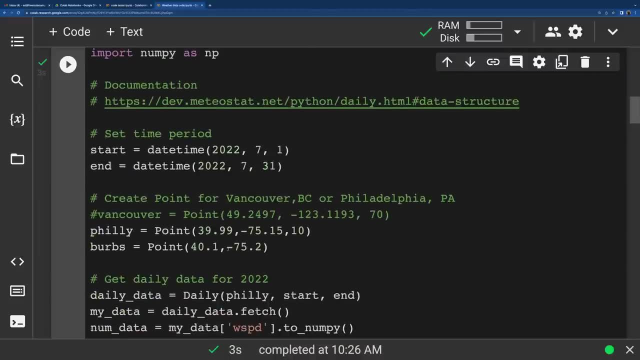 Yeah, we could take a look now I made this, so that's good and we can just pick that, and we can pick like any number of days, so I could, Since all the rest is already in there, I could just pick this and say, well, what about over the course of the year? 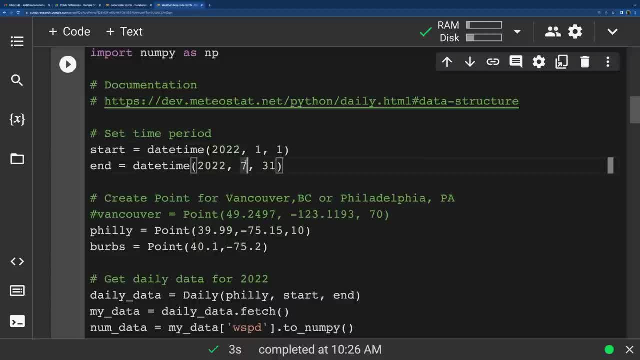 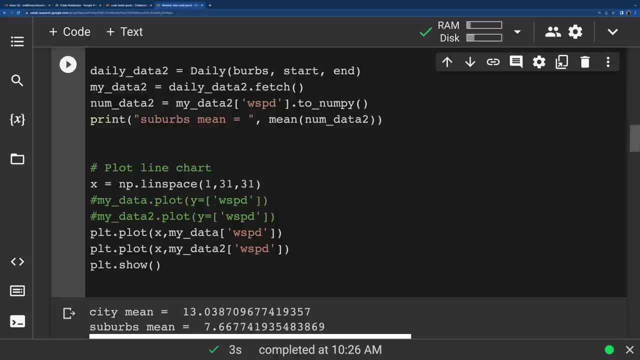 So maybe I make that like one one, and maybe I make that 12., 31. And There we go. so What if it would include? Then, There we go, So 365. And 365,. so I want to graph it this way: 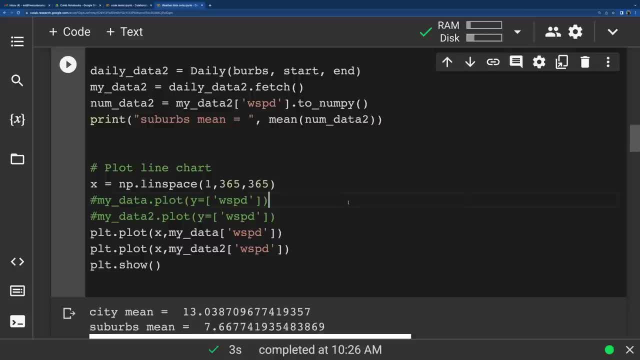 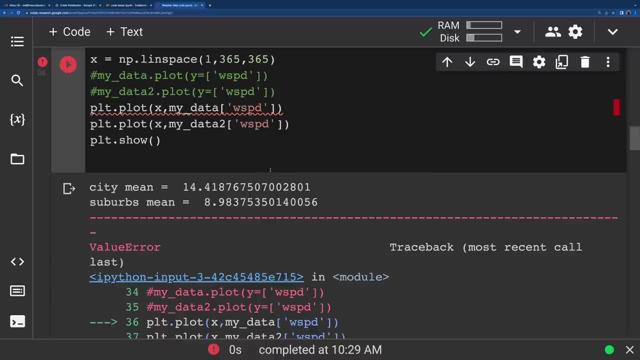 So from 1 to 365.. And 365.. If that doesn't line up perfectly, then I might have to do one more or one less, but we can take this and we can run this. Oh, value error, And it was. 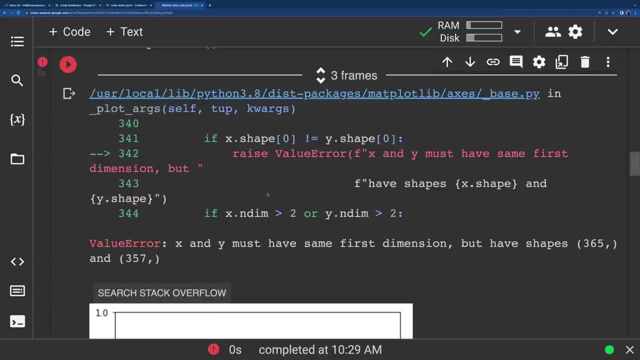 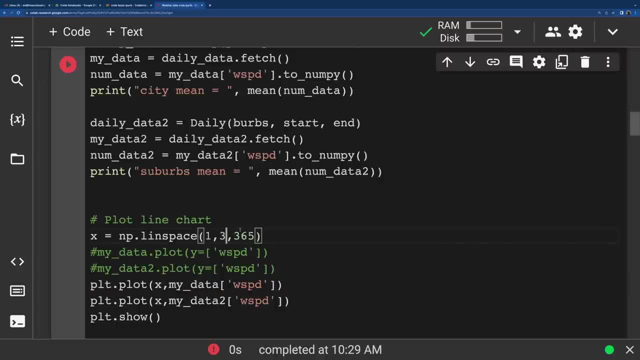 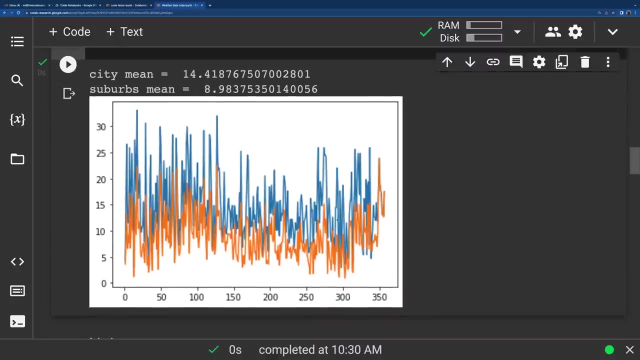 365, 357.. Oh, that's really interesting. All right, So 357. And 3. 57. And so we can see. you know the scattering, but also I liked this. Now why. 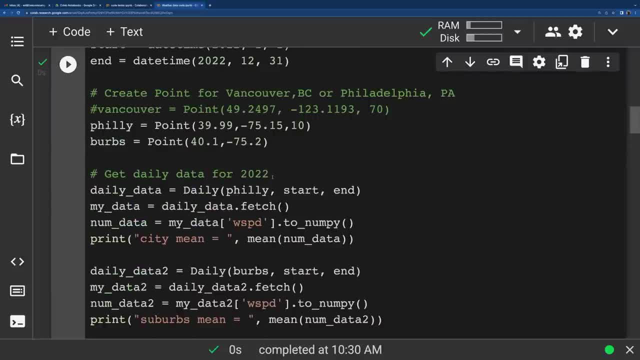 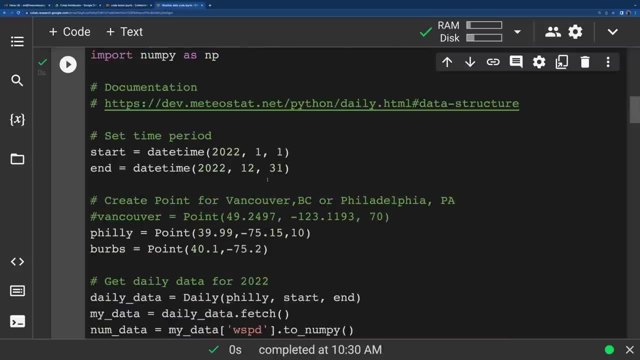 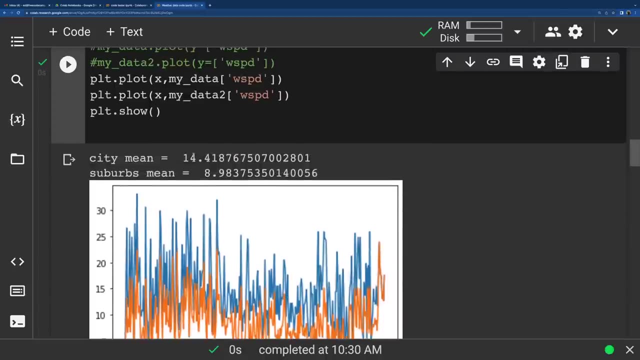 What? what I picked was, you know, not 365 days. That seemed like that would be it. I'm not really going to overthink that right now. Maybe there were some days that were missing, But you know, sometimes that happens. 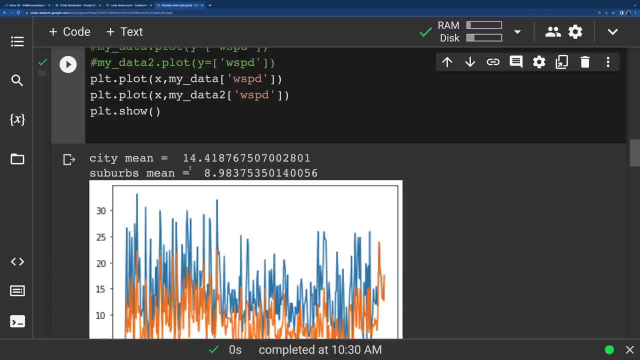 And we can go through and take out missing information or incomplete information. But now we take a look that over. So the day that I picked happened to be slightly lower than average, So in both it was up a little bit. you know, 14 miles an hour, 8 miles an hour. 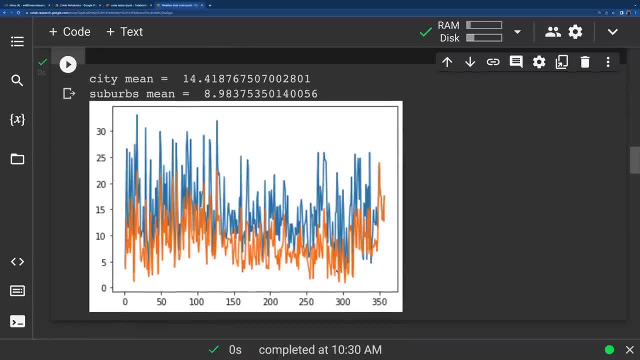 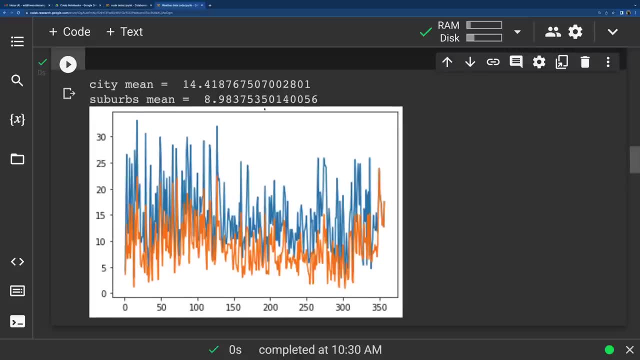 And then we can see the patterns here. So if this was wind speed, you know the average, then what you could do is you know you could calculate based on that average. You actually don't need to plot it out, because it works out given those averages. 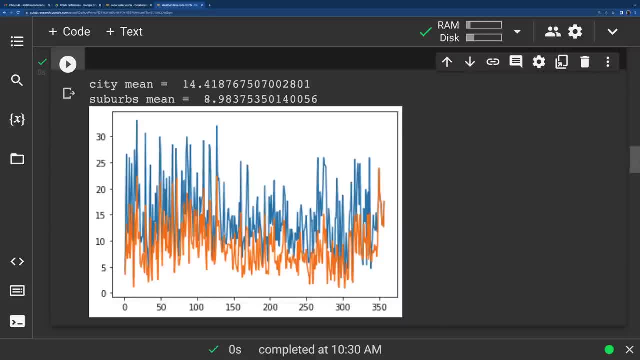 You can work on that. So if your wind speed is, you know, in the city and it's, you know, almost, it's like 14 miles an hour throughout the year, then you can look up well what size wind turbine. 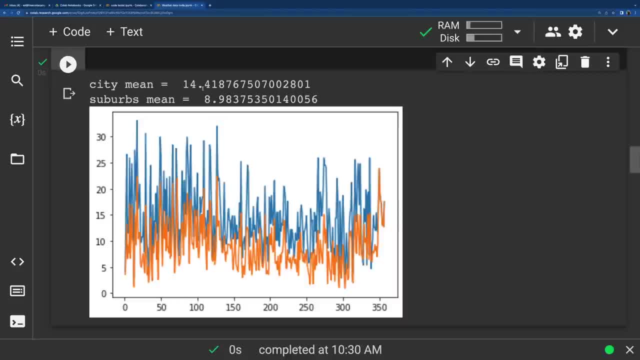 And it would be actually relatively small. But what size wind turbine you know would you need for 14 mile an hour winds And you can do some calculations. given that size of the turbine, How much electricity would that generate for you over the course of the year? 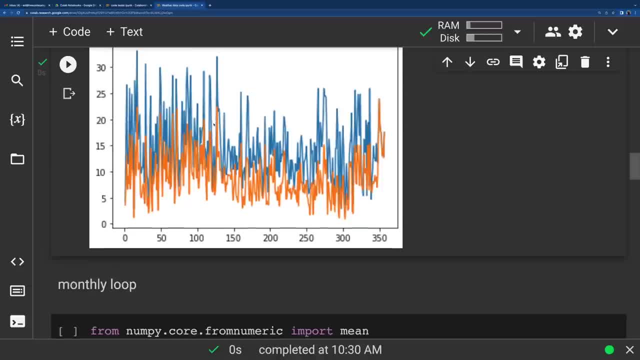 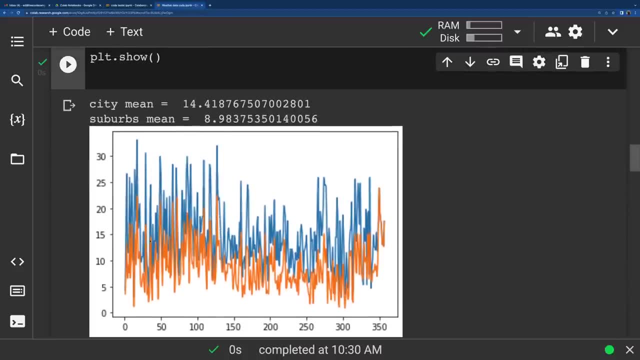 So pretty cool. And again, you can. you know you can do that with. you know any other aspect of this: The temperature you know. maybe you know you're trying to plan something, you know you can get. you know temperatures. 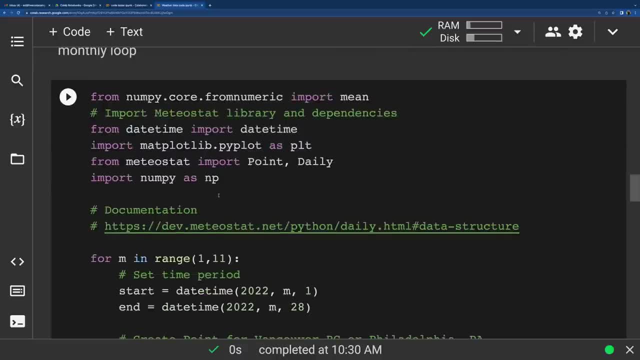 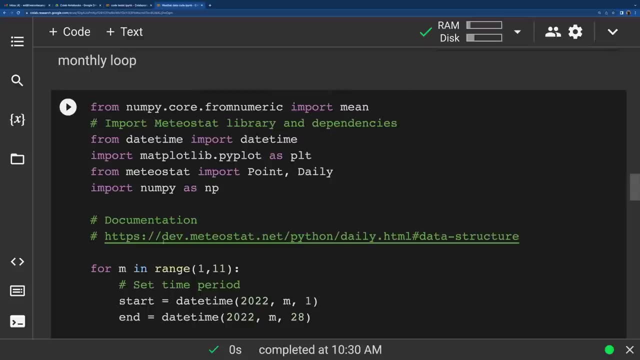 Just one other thing I did just was, you know, different. So I loop it through for you know, a month, just to show you. And all the rest of this is the same documentation link, And what I did is I just made it a loop. 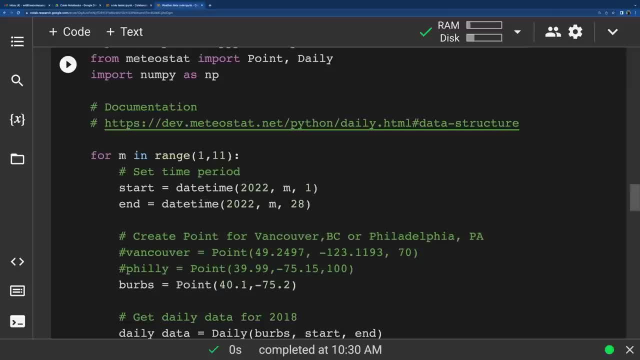 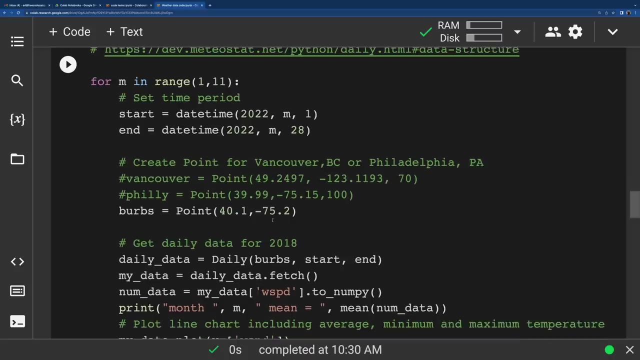 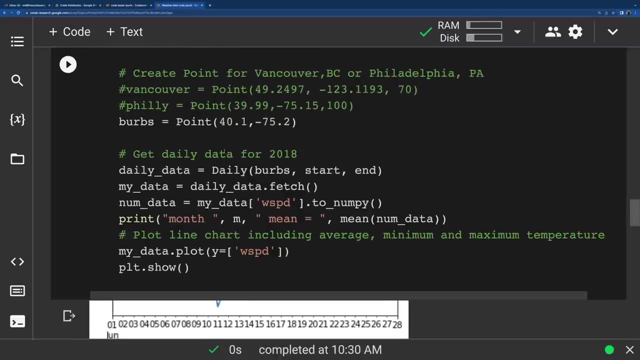 So you know, range 1 to 11.. And so that would be the month, And I have you know what month. There we go. And Yeah, there you go. I think I picked just this Because I thought: oh well, is that? 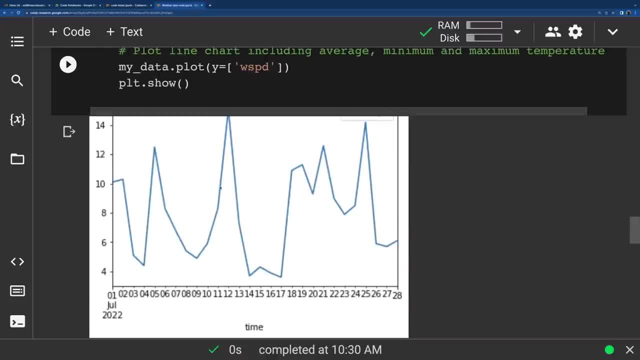 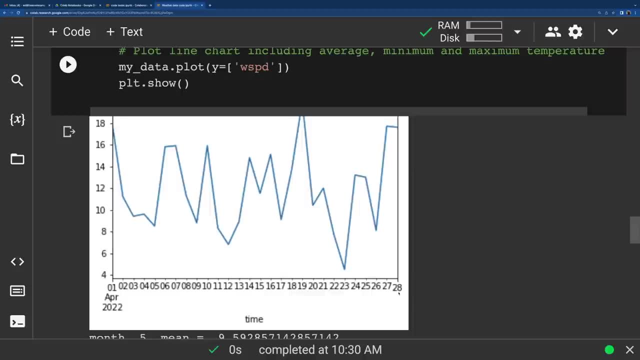 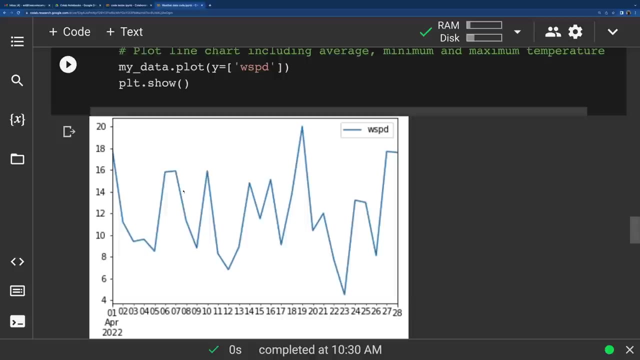 Does that change? And these monthly loops? Yeah, the way that the X value displays. sometimes it seems like a little cut off, But we can see we have, you know, wind speed And we can just see you know a few different months over the course of it. 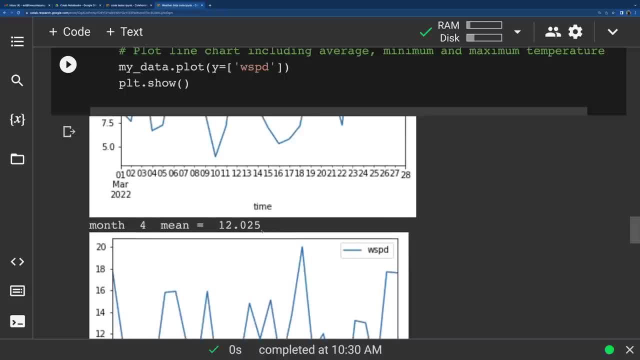 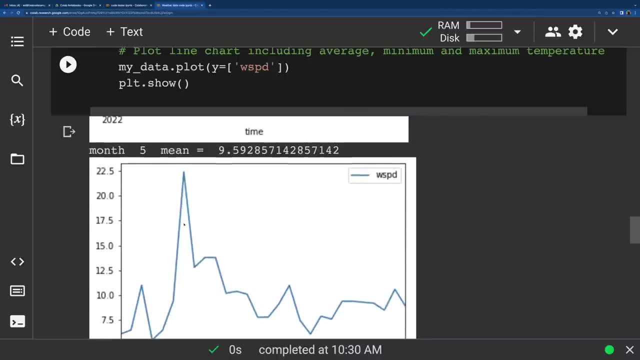 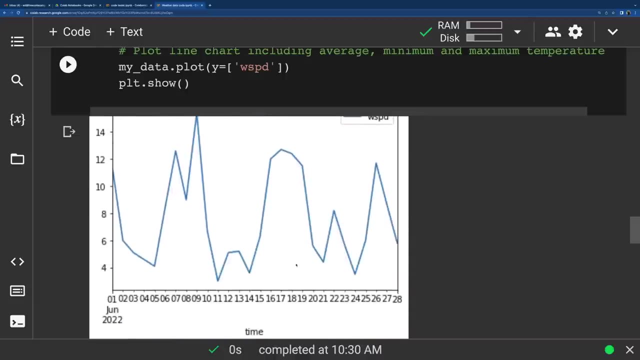 And you see, each month I have the mean And then And then the graph, So we can just see. It's just interesting. You know the mean and the graph for each month, The display. This might be a little clunky. 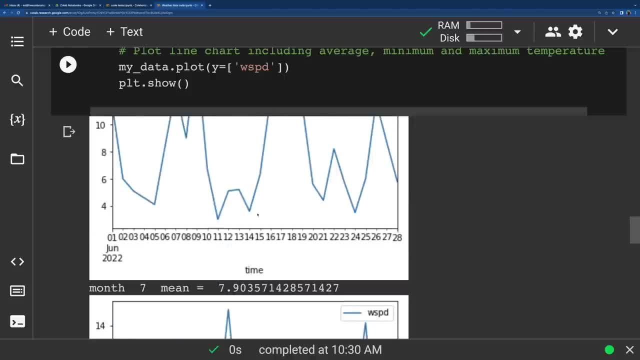 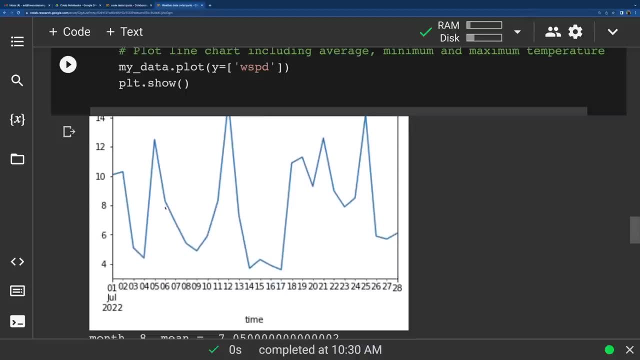 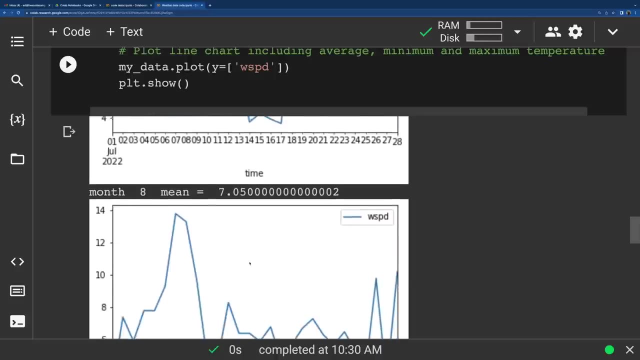 This might just be for your own interest, Or you could have something that displays them all in some nice little you know 3x4 grid. It gets to be small graphs though, But nonetheless We see. We see that there's times when it goes down. 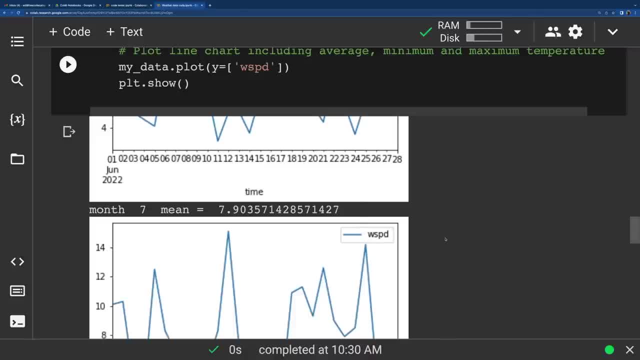 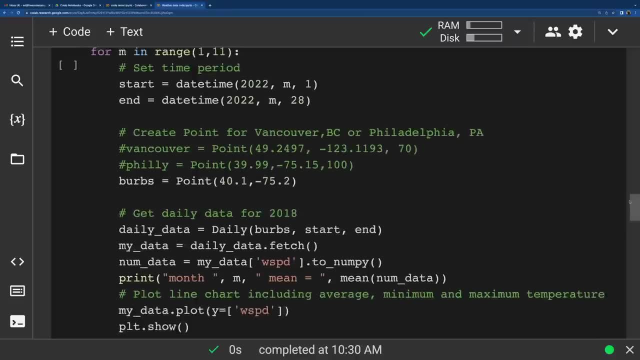 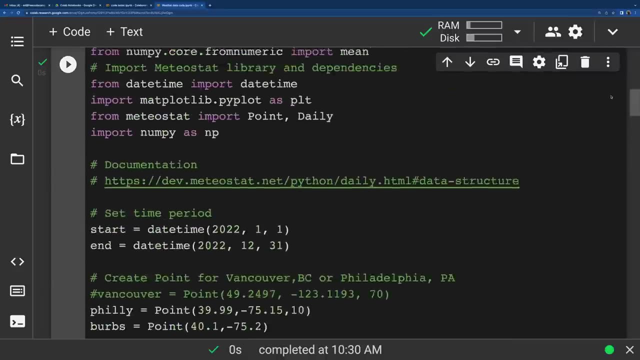 So I just wanted to show you some of these things that you can do with this graph, And you know beyond that that there's other ways And what you can do in you know any other data you find, And if you know you're looking up some things, you might find them. 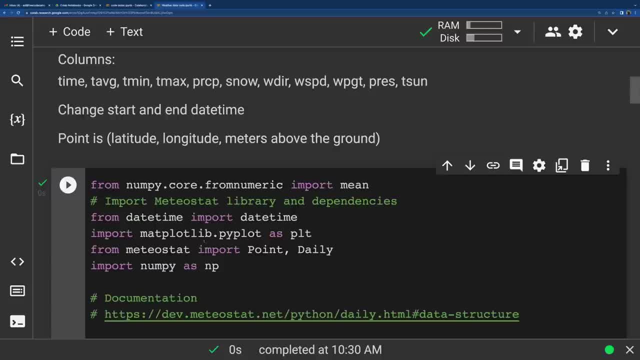 Maybe it's a CSV, But maybe somebody you know put together an entire library And with that they not only have the data and then that's stored somewhere. But you know, somebody also wrote these functions so that you have all these already. 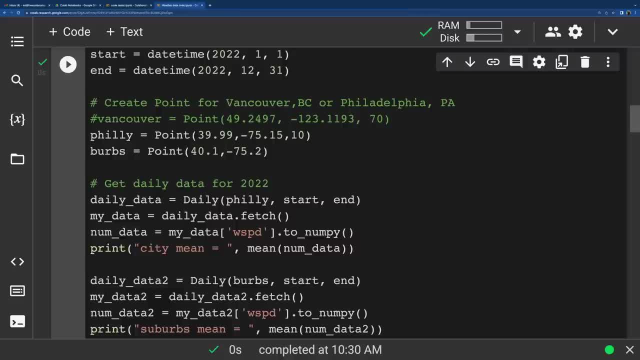 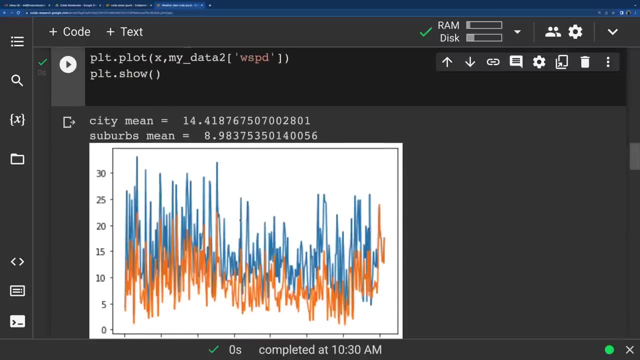 How can I get a point And how can I get all this different data from any of those points? So things that you can make and things that you can find online that somebody else made. You know Different ways that you can find this data and then graph it. 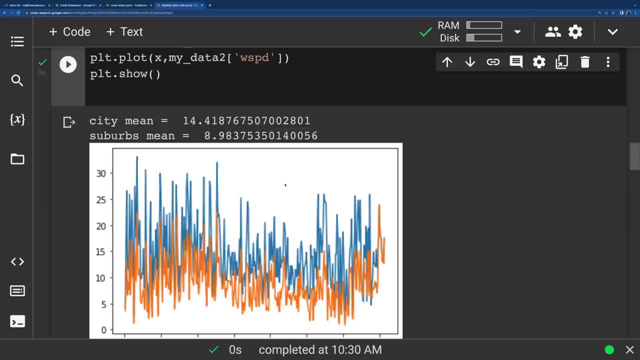 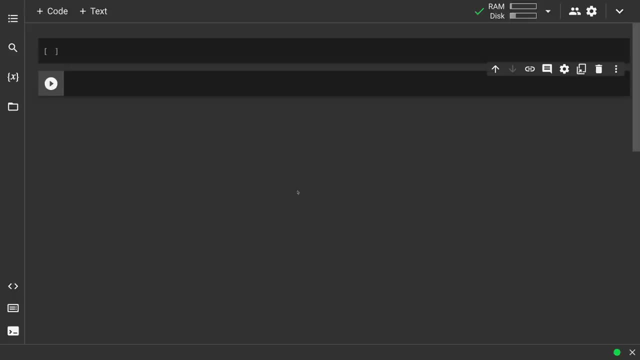 So trying to give you some more tools. Now that you know math and Python and can use this to graph, you know some more tools and some more sources of data. So what I want to show you here is just a few more things that you can do right within Colab. 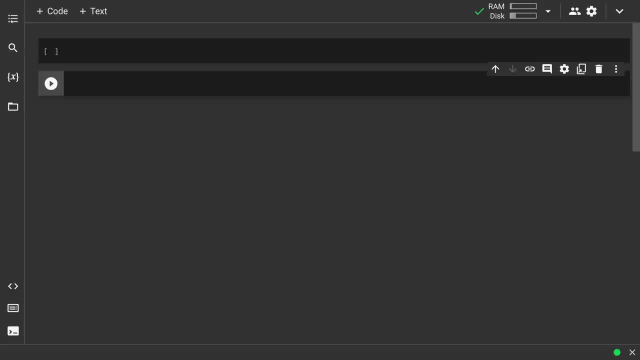 And we already looked at over here on the left The Table of contents that you can get to appear or disappear. Then we have the search. You can even search for directly for variables here- And then we have this folder icon where you can click to mount your Google Drive directly. 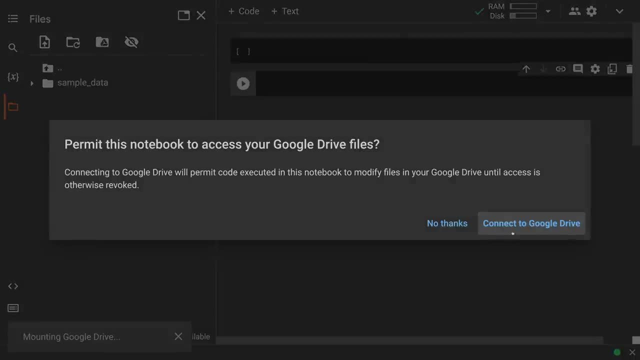 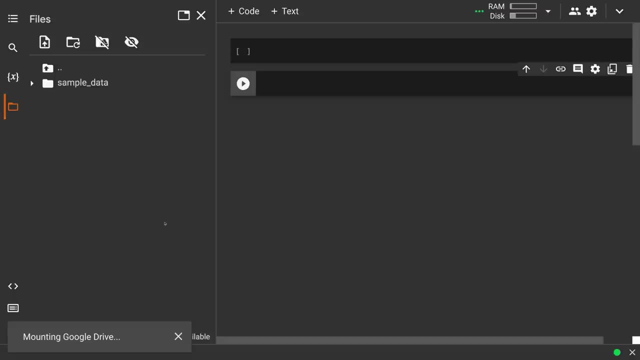 And then, once you do that, then you can also see give it permission And down here we see it's mounting the Google Drive. Once you do that, Then you'll see it has the slash through it now so you can unmount the Google Drive if you want, if if you wanted to do that. so this makes it easy to find things and move things back and forth within your Google Drive. 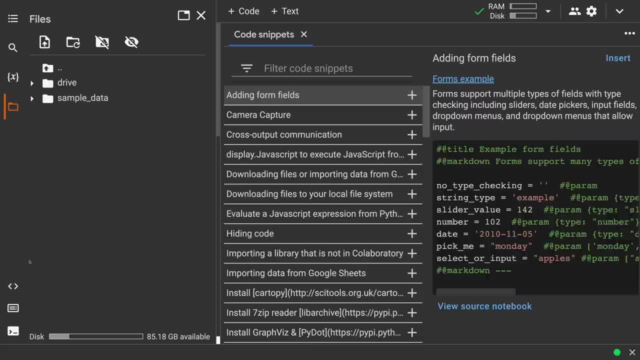 Then the really big thing down here is The look at these tags. you can get all these code snippets that are already in the Google Colab, say, adding form from fields. Oh, I want to add a form. If the code right here, you can copy it or even click it. you know, if you happen to be right in the place where you want to put it, you click, insert all these other things, camera capture and notice this even. 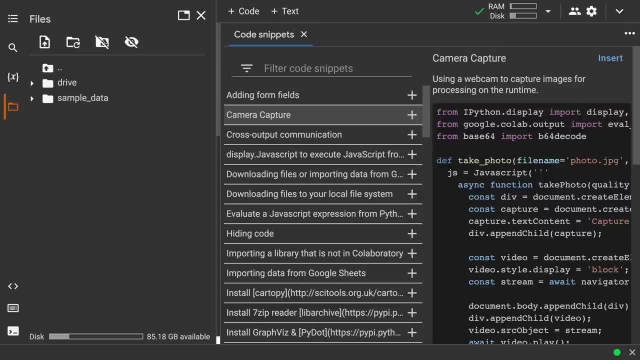 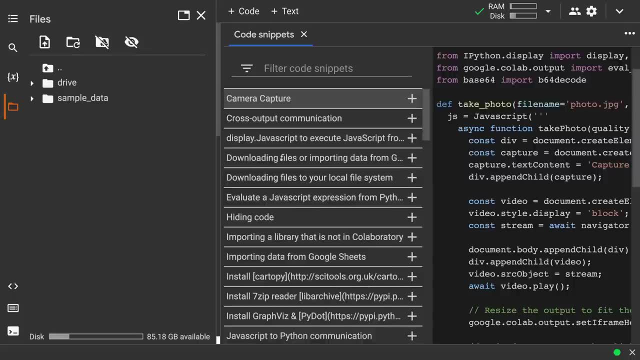 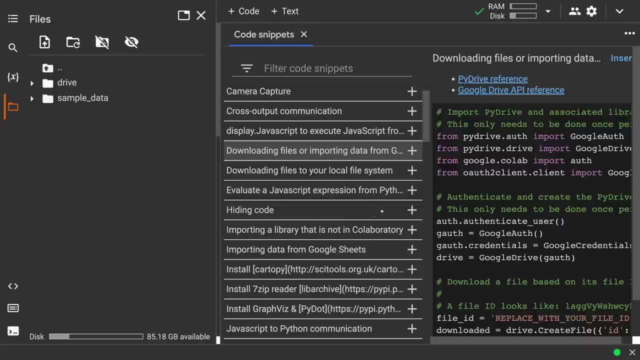 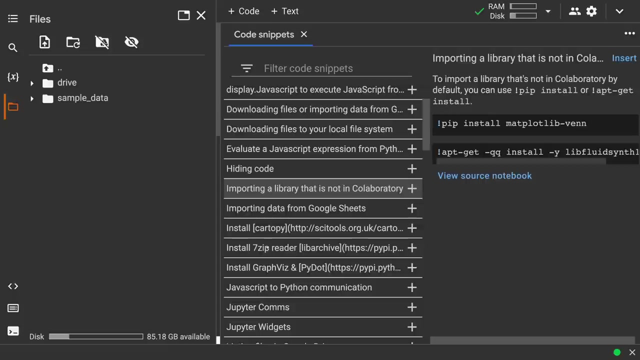 Uses JavaScript within Python interfaces, this. so it's pretty cool Again. all these And some of these you know, downloading files From Google Drive, From GitHub, all kinds of things, Importing libraries that You know that are in Baseline, all of these zip reader. 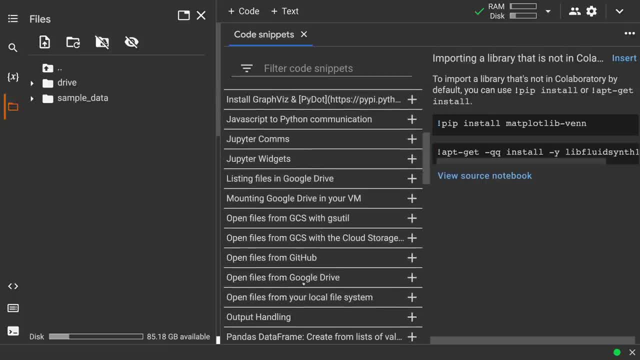 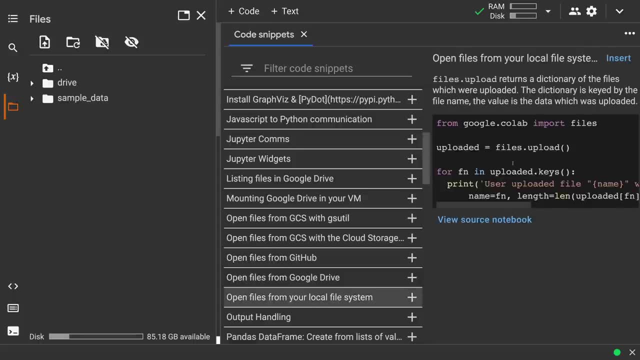 There's a lot of other things You can do: open files from GitHub, from your Google Drive, from your local file system, How you can just upload those So And even gets down in here into Pandas Data free, And that's kind of where. 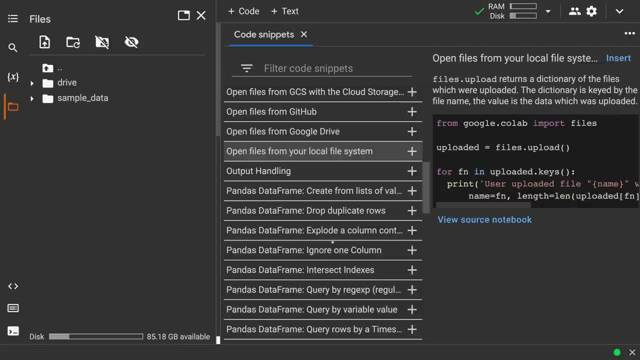 We want to get Our math skills too. Get our math skills, And that's kind of where we want to get our Math skills. consumer data, web resources, too. We can take data from wherever- Well, that's the pandas part- and then bring it in and then do. 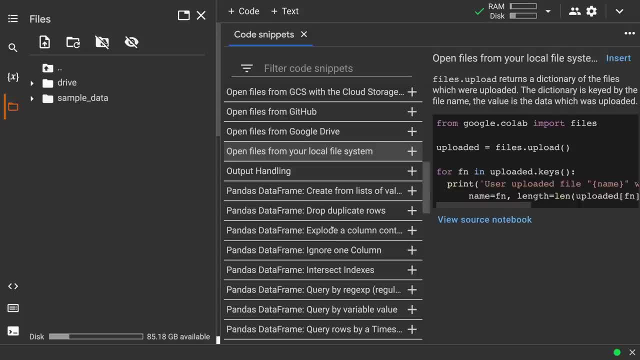 some different math to it. What can I graph? Can I display it in different ways? And that's what we want to take this to. So what I'm going to do is you'll see below this video. there's other code that I'll include, but I'm not going to go through every one of these, but check these. 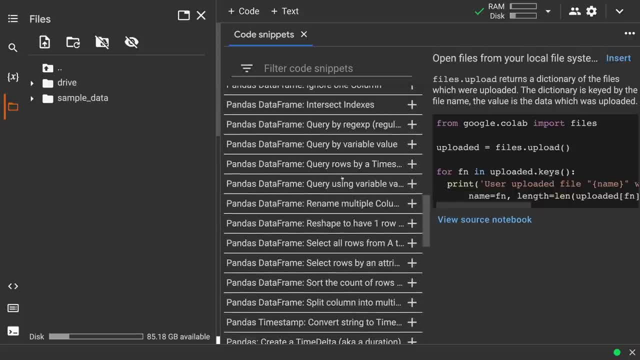 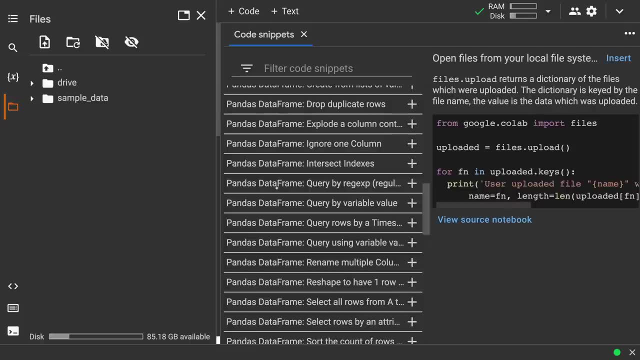 out. I mean, there's so many different things already built into Colab that you can do, Open up a sample and tinker with it. I have a Colab notebook- I just call a code tester- and I just have different things that I can go through and let's try this, let's try that And 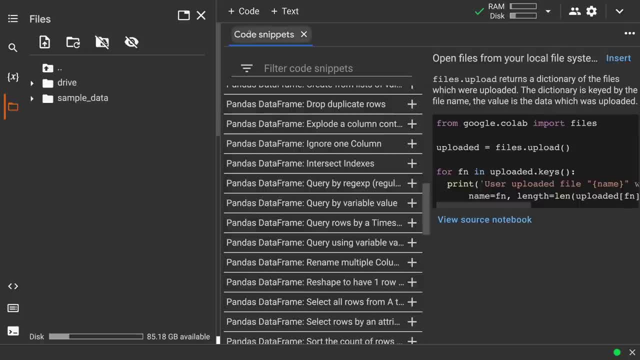 then you put together in your notebook of stuff that works- But here's all these things available. and then I'm going to put together another Colab notebook of just a few other things to tackle on this end of the scene, And then I'm going to put together another Colab notebook of just a few. 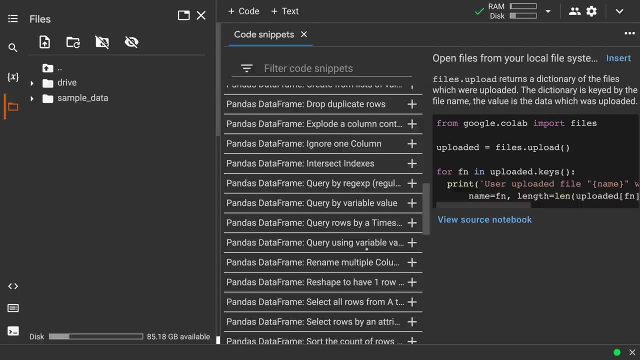 things to tackle on this end of the scene, And then I'm going to put together another Colab notebook class to continue some things that you can do with math and with code, And we're building upon this, leading to working with data and doing some other interesting things with that. So 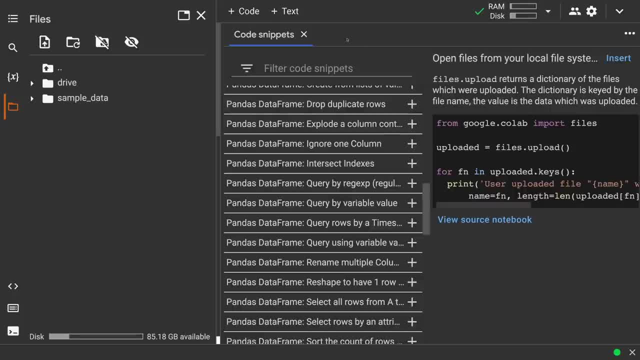 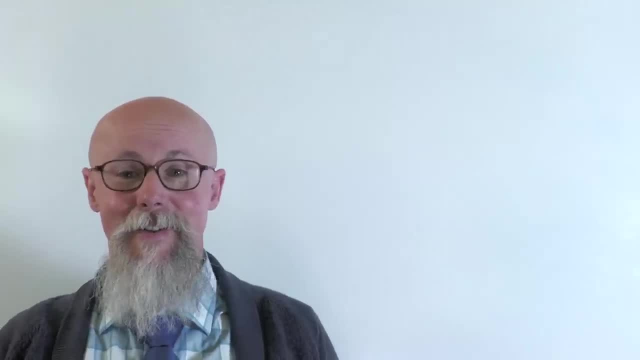 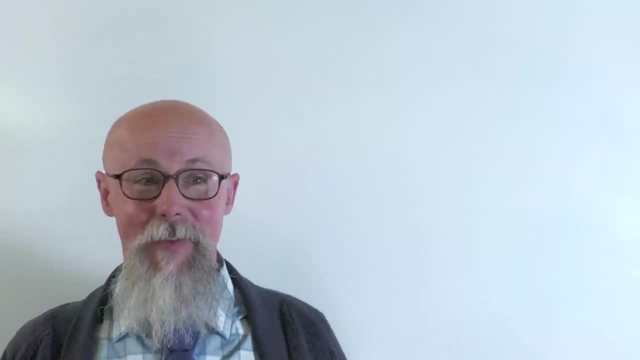 check these out and tinker with them and enjoy. Wow, you made it So now, having gone through this, now you should have a good understanding of algebra. You should be familiar with all the key concepts and how to write the code to do all of your algebra You should have. 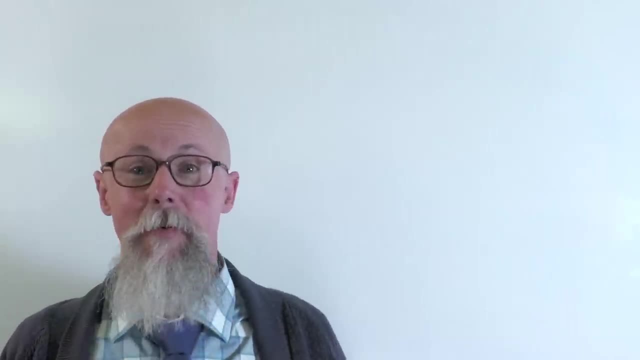 your at least one- or however you organized it- Colab notebook that's ready with all of your scripts for solving all different sorts of algebra problems. You made it through certification one, two and three, And you have the ability to solve a lot of different.